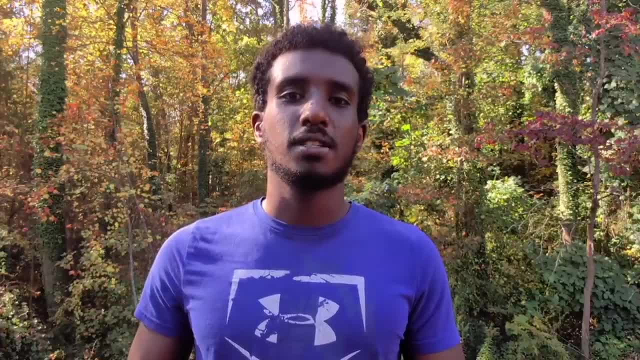 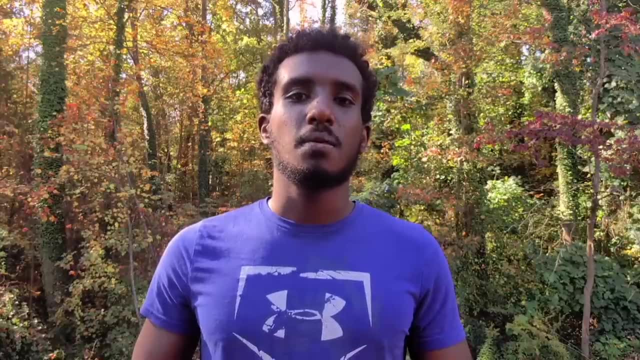 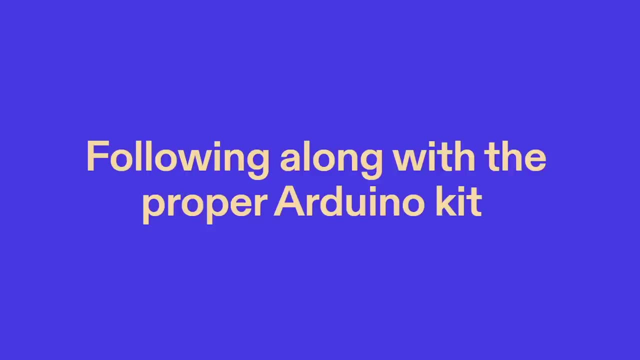 kit, as it is more engaging, but I will also be using a physical Arduino to teach. But if you don't have one, don't worry, I will show you how to follow along using a simulator. With that in mind, let's start our first section Before even working on a physical Arduino. 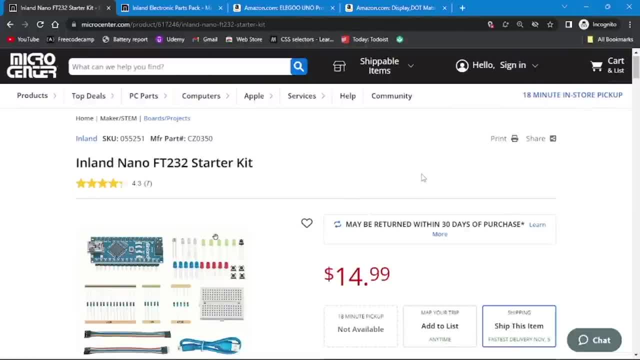 the first problem that we run into is there are thousands upon thousands of Arduino kits. We do not know which one to use to follow along in this course. In this course, I'm going to be using an Inland Starter Kit and an Inland Electronic Parts Pack. 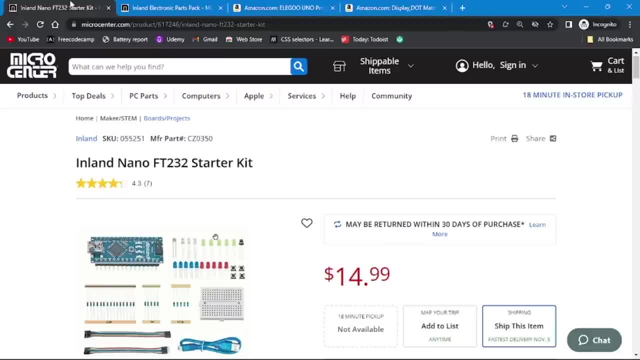 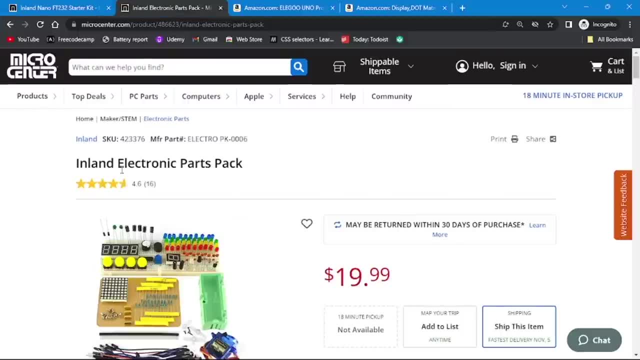 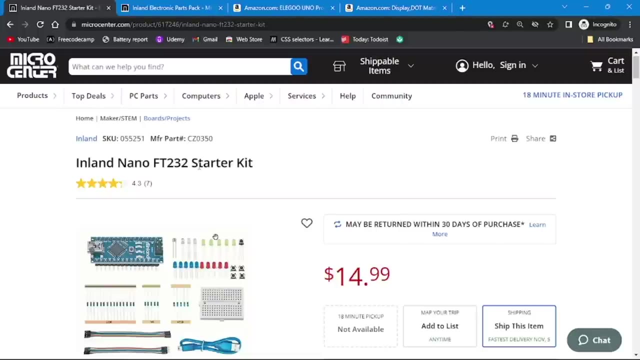 I'm going to leave a link in the description of this video so that you can check it out for yourselves. Okay, so I'm going to be using an Inland Starter Kit and an Inland Electronic Parts Pack, But when it comes to these Inland Starter Kits, they're mostly available in 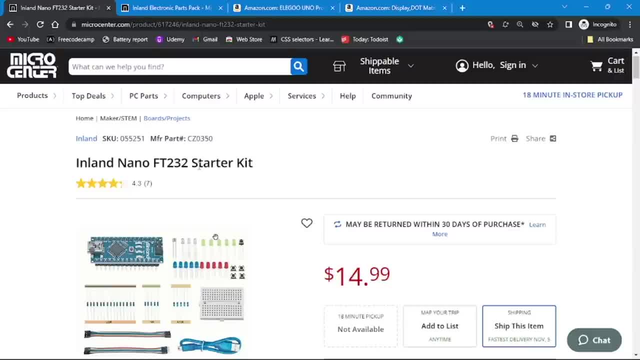 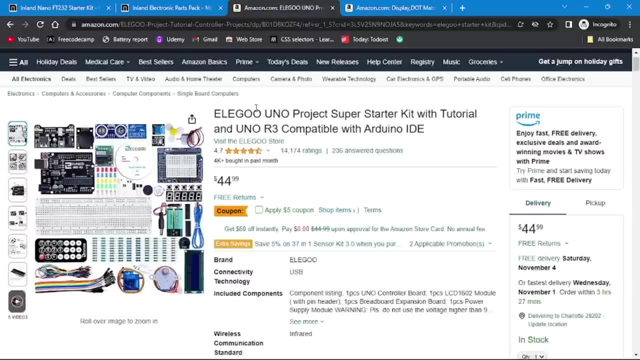 what they're only available in the us. so if you're outside of the us, you can get yourself an elego uno super starter kit. okay, you're going to get yourself an elego super starter kit with an led matrix, so this kit does not have an led, a component named led matrix, which is very important. 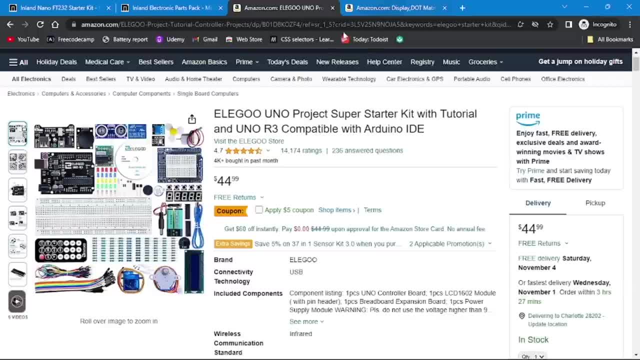 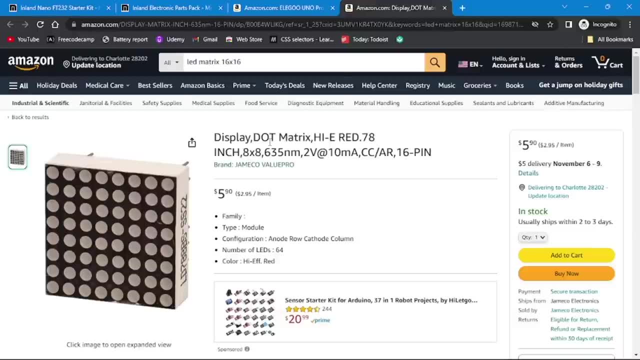 because i'm going to be using it in this video. so you're going to get yourself an elego super starter kit and then you're going to get it separately. you're going to get an uh display matrix- okay. so an led matrix- okay. so one final thing is: if, let's say, you already have an arduino, 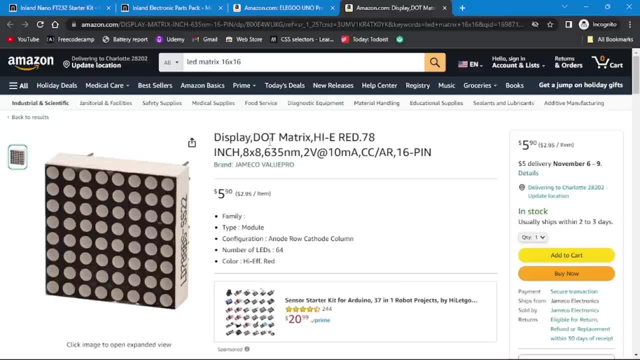 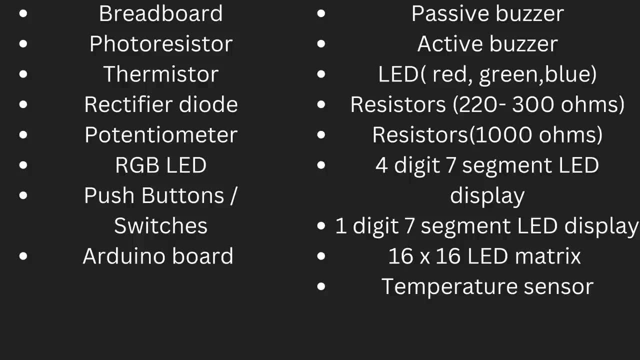 kit and you want to know all the components that i'm going to be using in this video. i'm going to see them on the screen right now so you can again cross check on your arduino kit and on the screen right now. if you have the kit, if you have the components that are required. if you don't, you 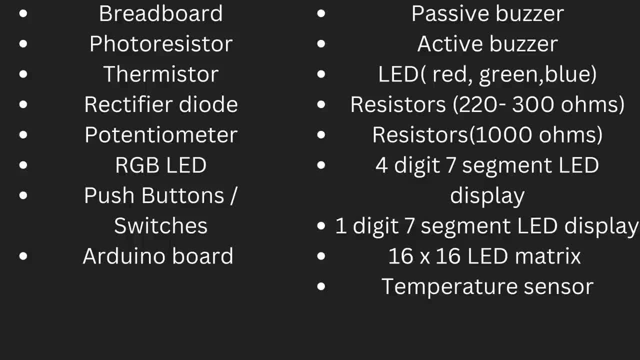 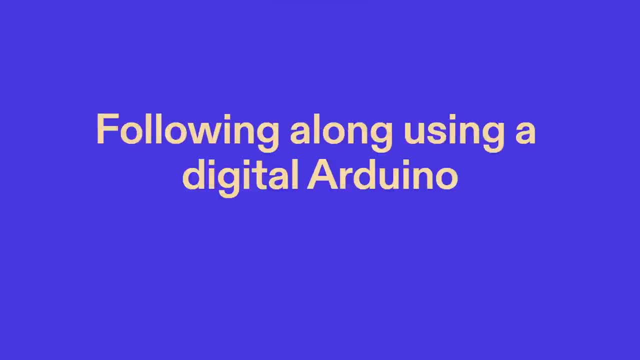 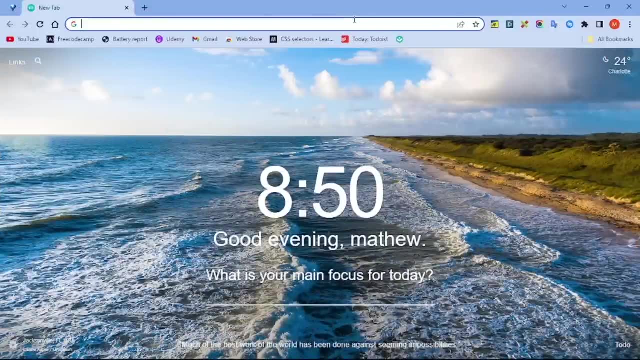 can again separate them out, and then you can get yourself an elego super starter kit and then you can separately google them and try to buy them from amazon and different stores. so with that in mind, let's move to the next section. okay, so for those of you who don't have a physical arduino and want to follow along, 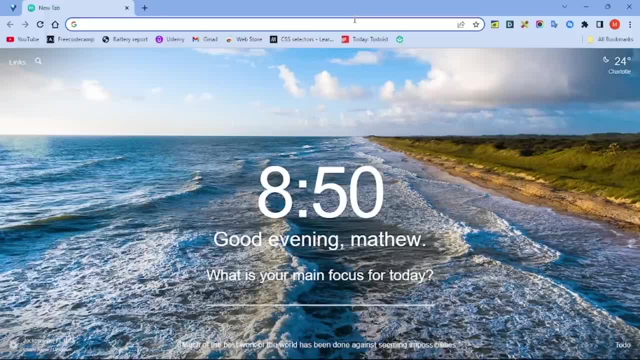 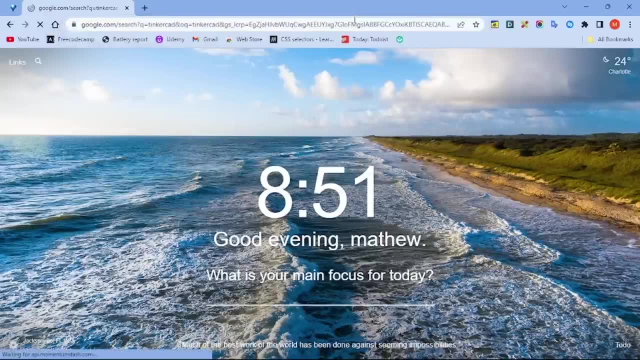 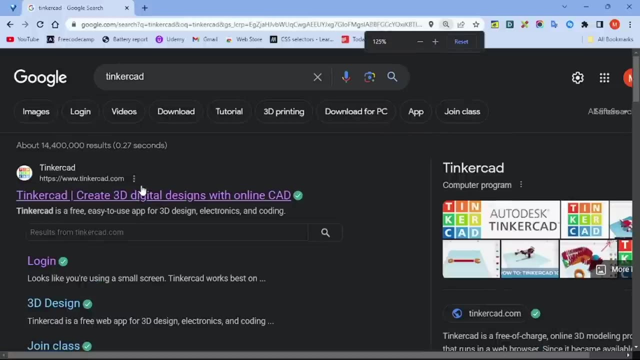 using a digital arduino. i'm going to show you how to do that. so what you're going to need to do is go to your browser and then go to tinkercad and then touch the first link. it's going to be Tinkercadcom. Let me just zoom in so you can see it. There we go And then open. 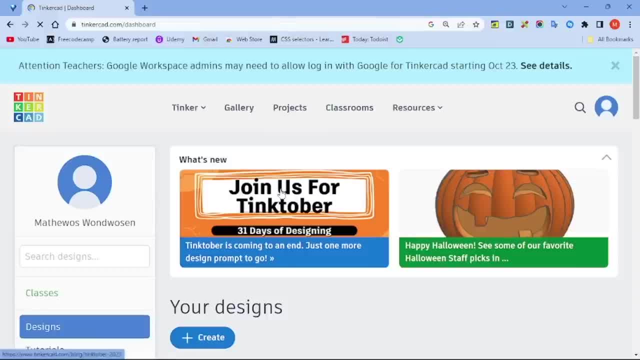 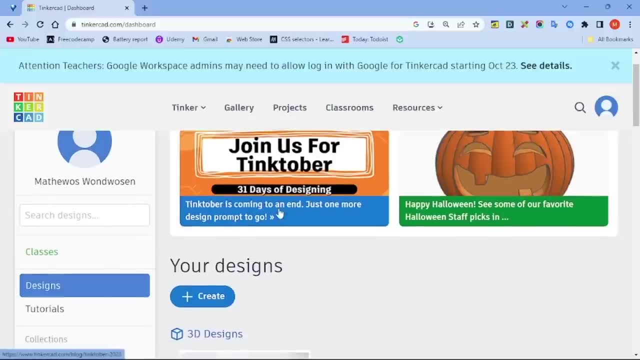 it Okay. So for those of you who are joining or using Tinkercad for the first time, it's going to be asking you to sign up or log in, So we're going to do that. I already use Tinkercad, so I'm just 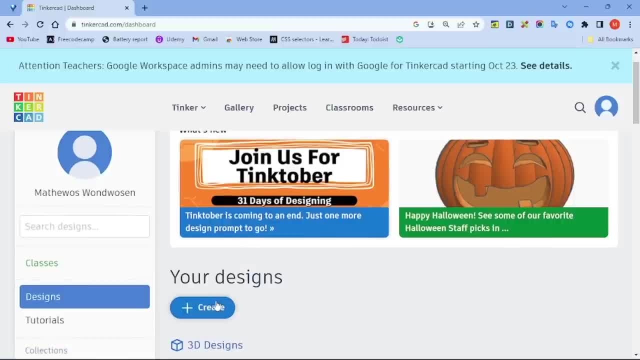 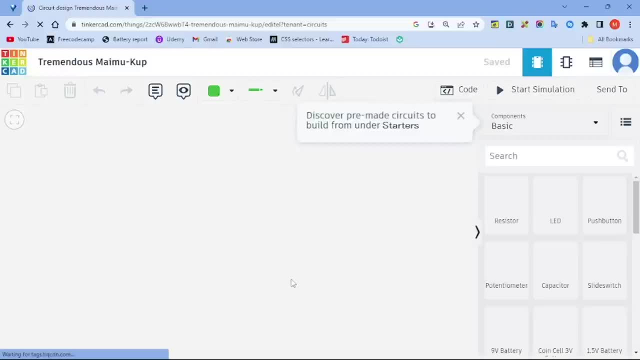 going to log in directly to my account Afterwards. all you need to do is go to your designs, create one and then go to circuit And it should be loading. And once it's done loading, all you need to do is use this tab for components. So you're going to be searching for the components that 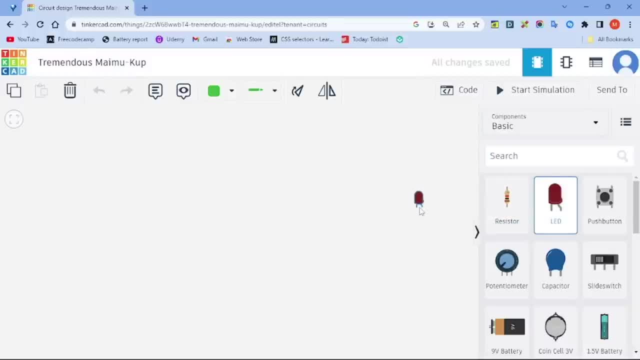 you need right here, and then tapping them and adding them when you do, And there is a code section right here. So basically you can write code to your Arduino and then you can start the simulation. That's all you need to do to follow along using a digital simulator. So with that in, 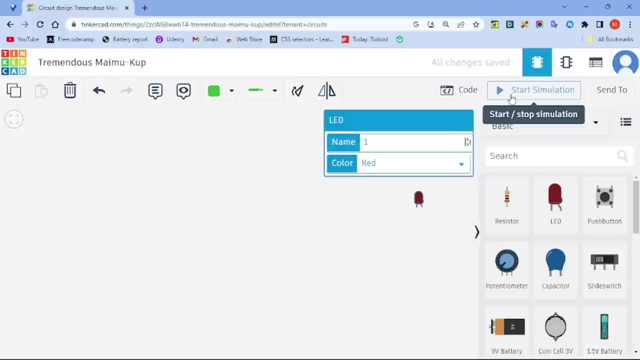 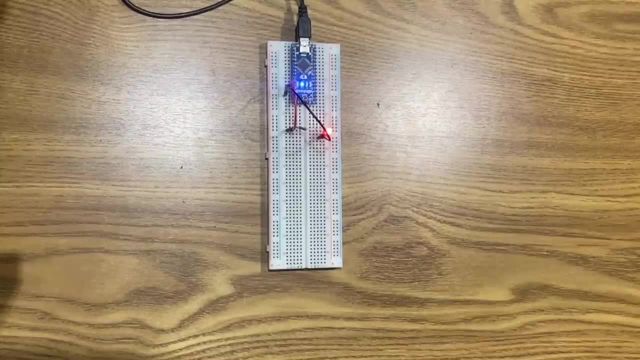 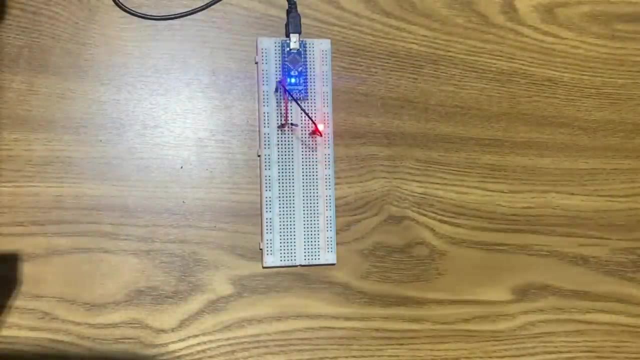 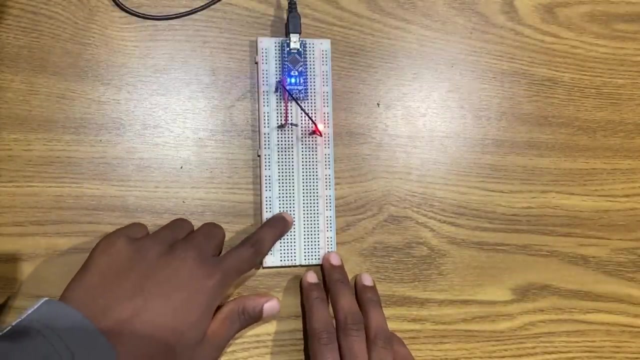 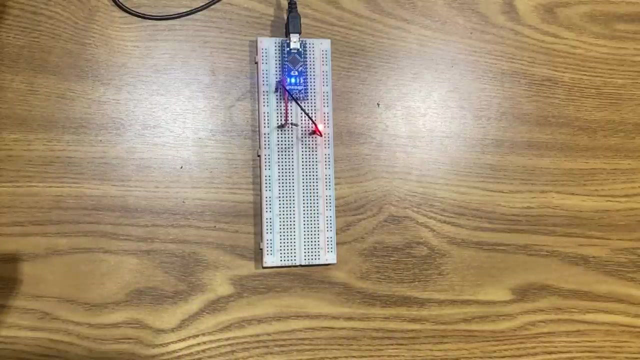 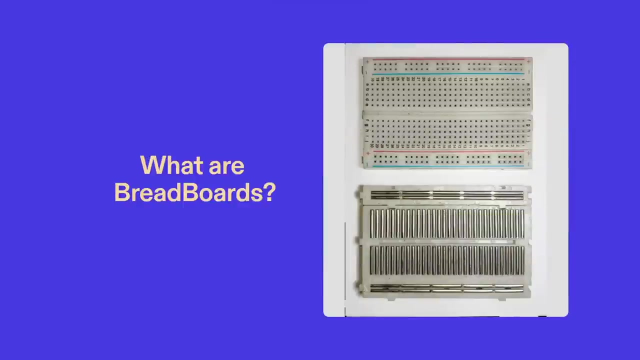 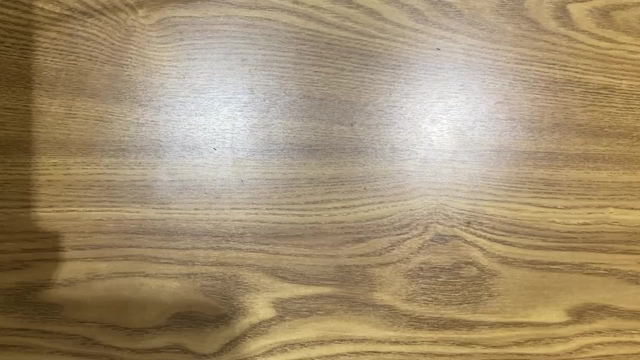 mind, I'll see you in the next video. Let's actually work on our first Arduino project, Assembling them into this one project. So see you in the next section. Before actually talking about web boards, let's say I want to connect my Arduino and build a. 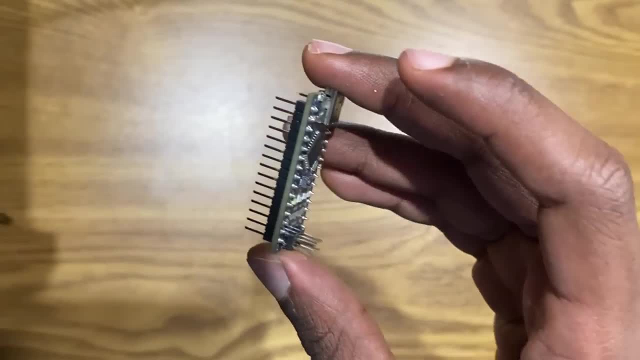 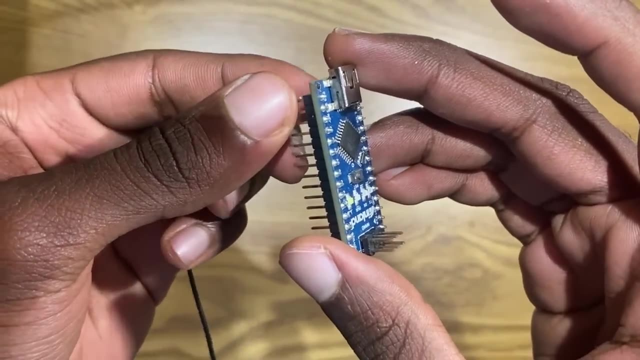 simple circuit. Okay, I have my Arduino right here And before turning it on I'm going to connect the pin. let's say right here randomly again Say I want to connect it. I'm struggling a bit right now to hold it, Okay. 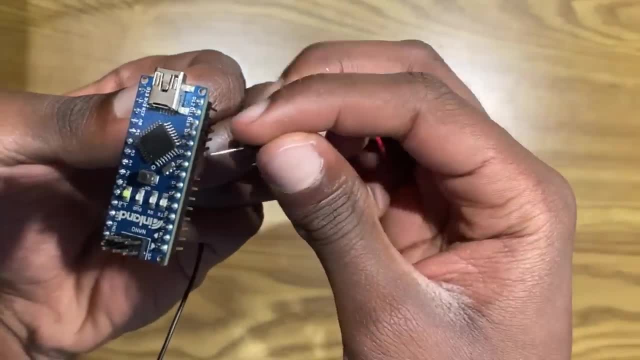 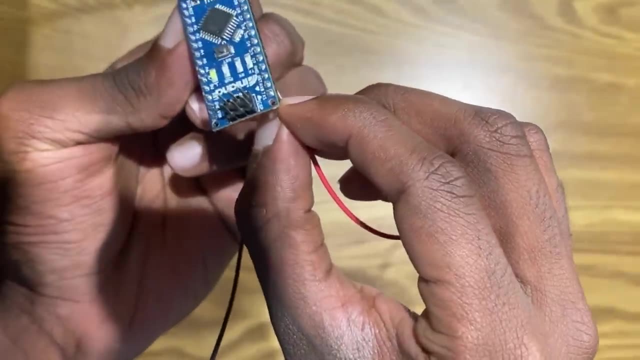 It did hold it. It's a bit of a struggle. Let's say: I connect, connect it to here, It's not even comfortable. Let's say: connect it to here, Okay. Then let's say: I'm going to use a third wire, I'm. 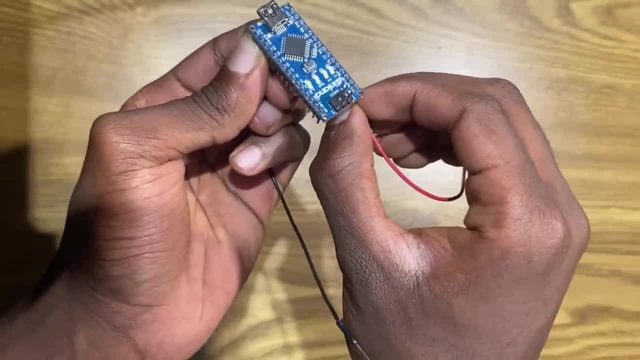 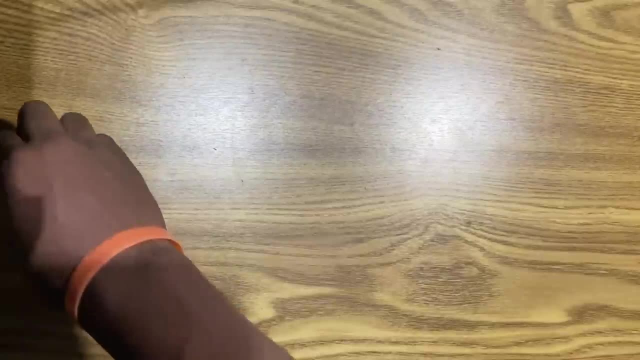 going to be building a complex circuit. In this case my hands are preoccupied, So I cannot really build a more complex circuit, as, again, I cannot put a third wire. So this is where web boards come in and actually solve the problem. Not only that too. 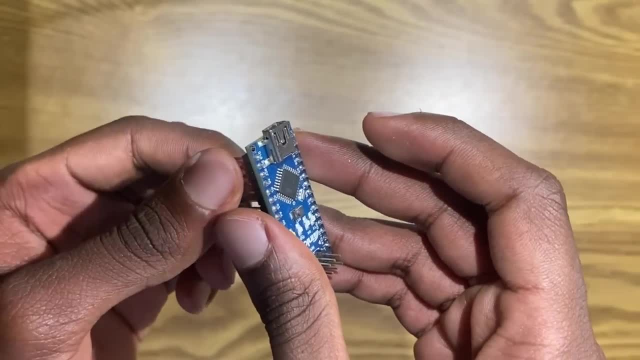 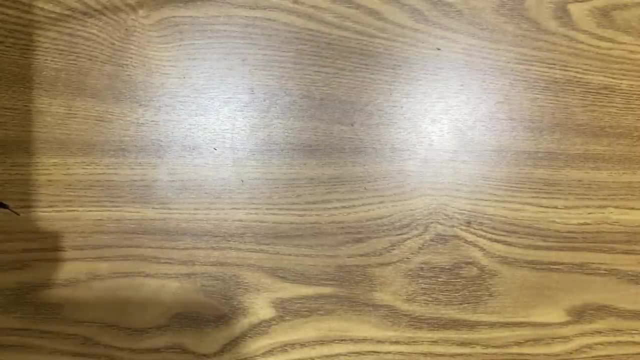 But also, if I turn on the Arduino and I, as I said, again connected to the pins, I'm going to be zapped. I don't want that to happen. So now I'm going to bring my breadboard right here. 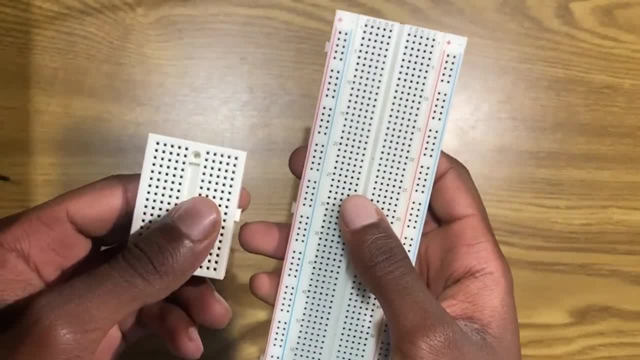 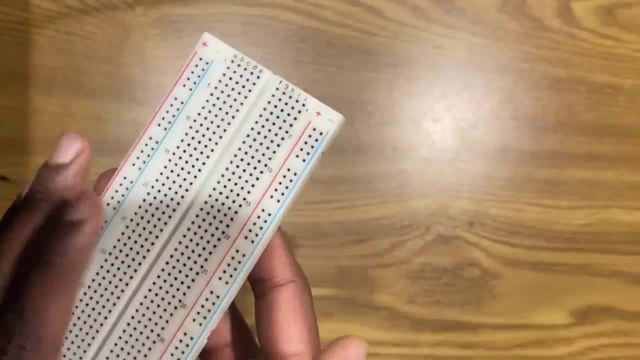 So breadboards come in different sizes and different shapes, So there's a smaller one and this is the bigger one. I'm going to be using the bigger one to explain what are breadboards and how they work, So I go real close up here. Let me just point my light towards. 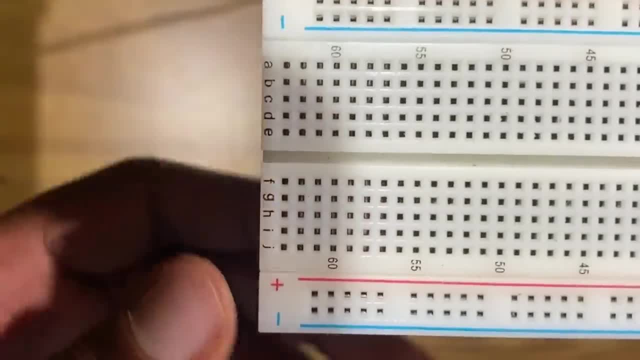 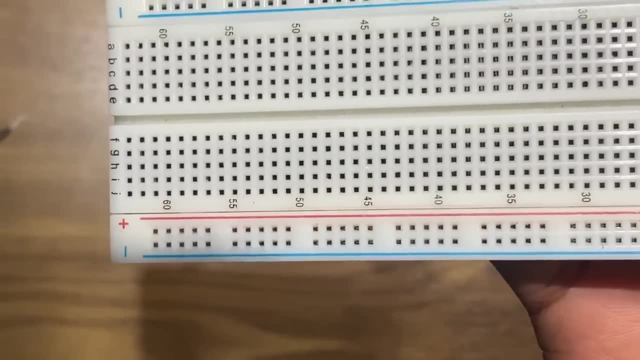 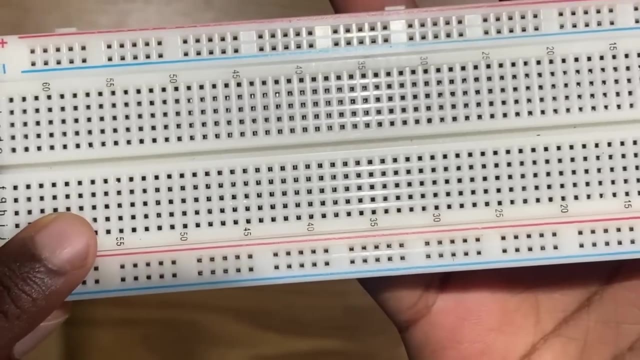 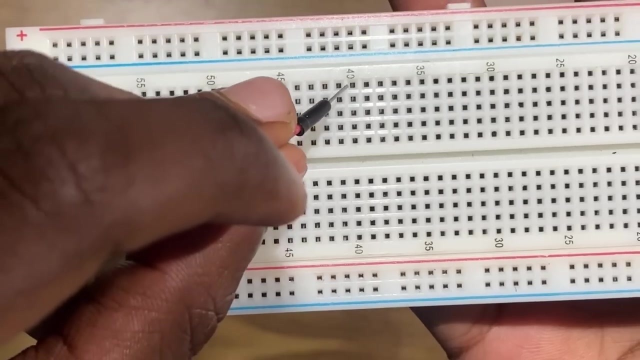 this so you can see it. Okay. So if I go close, really close actually, Let me zoom in. I zoom in right now. And if you check this out, is you see wires that run horizontally? Let me again. Okay, There we go, We can see it right now: Wires that go horizontally right here. All of that You can. 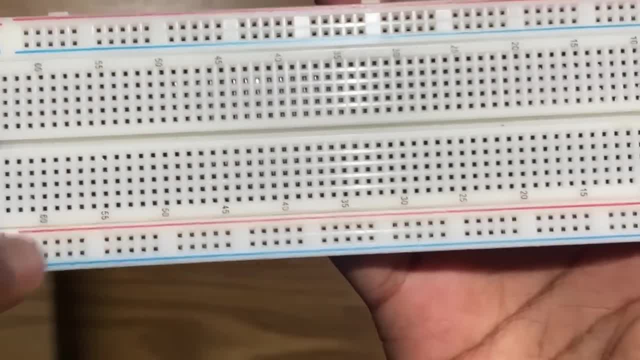 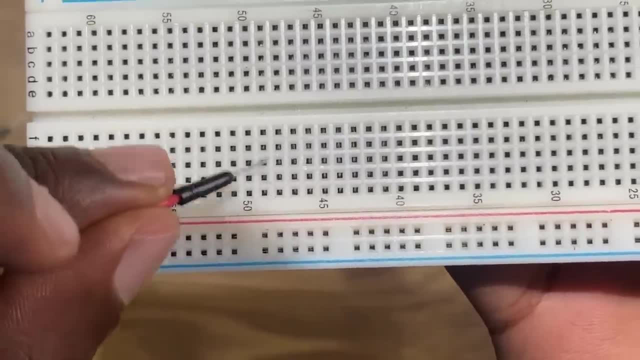 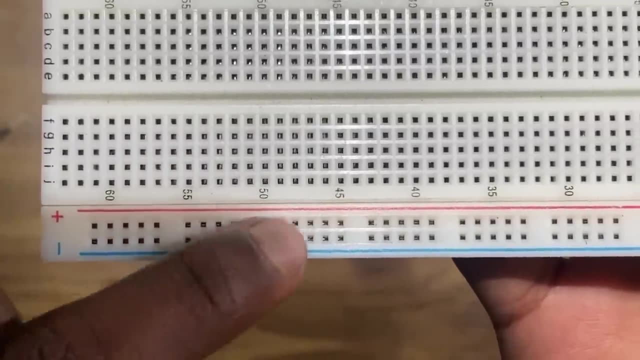 see that there are wires that are going horizontally. Okay, The same goes for this one too. I can bring it up close towards the light. Okay, There we go. They go horizontally. If you check them right here. if you look at these two wires right now, they go vertically. Okay, The ones. 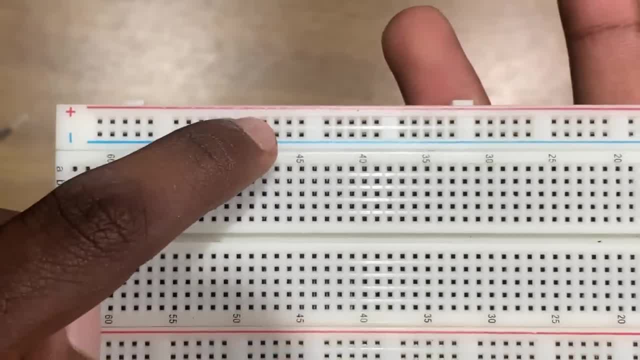 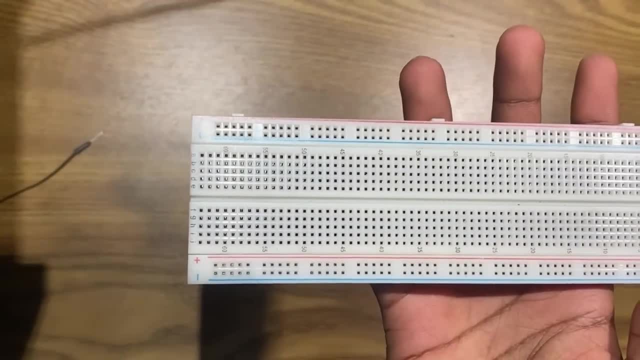 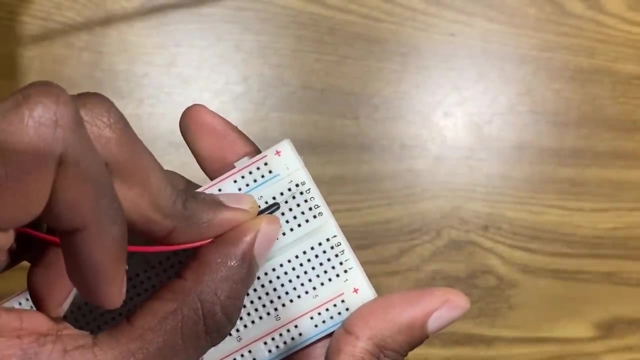 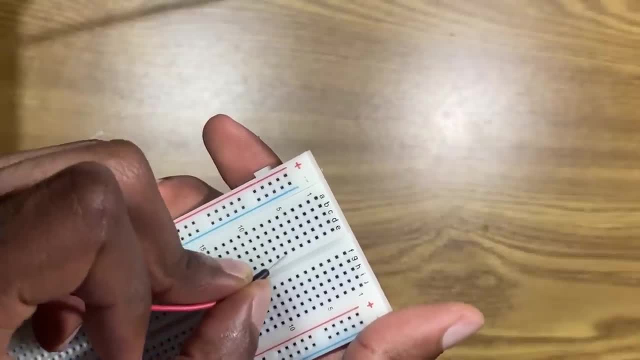 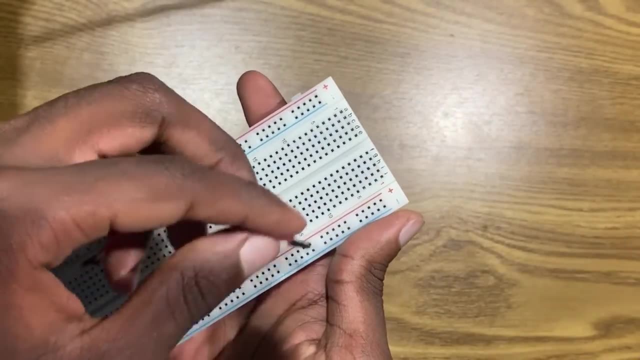 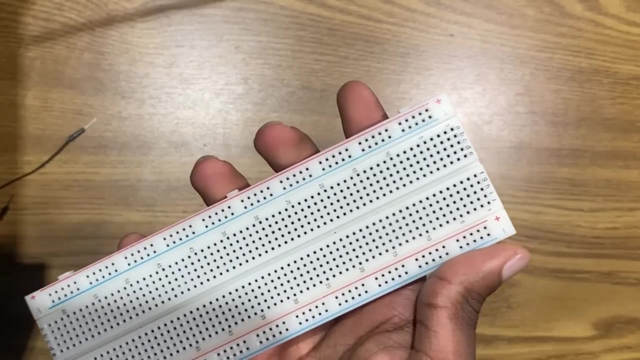 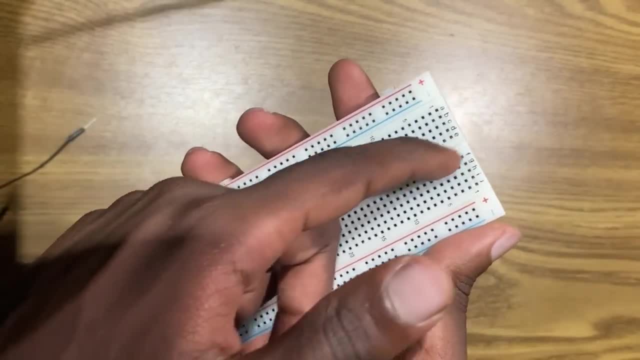 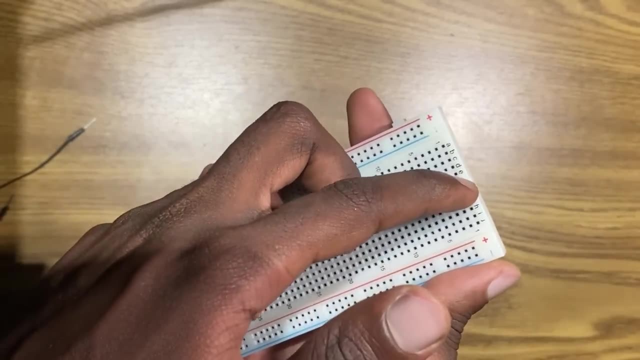 thing is E and F are not connected. Okay, There's a gap between them. As you can see right here, there's a big gap. There's a gap between E and F. So one thing is: E and F are not connected. Okay, So A up to E are. 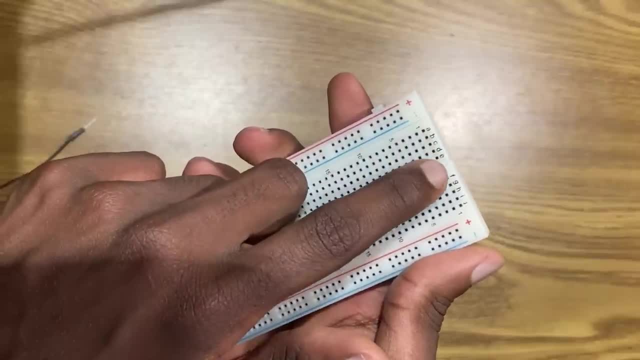 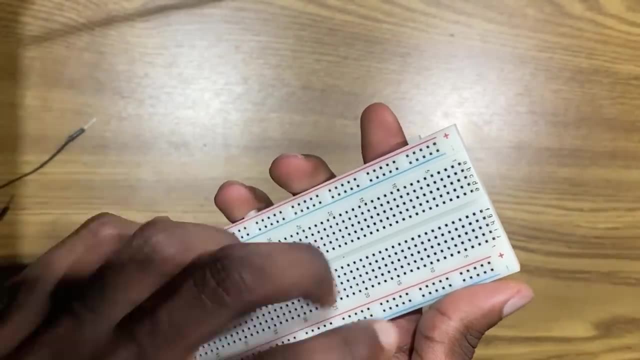 connected on their own, but A up to E are not connected to F up to J. Okay, So they're not connected. A up to E is not connected to what: F, G, H, I, J, basically, So they're not connected. 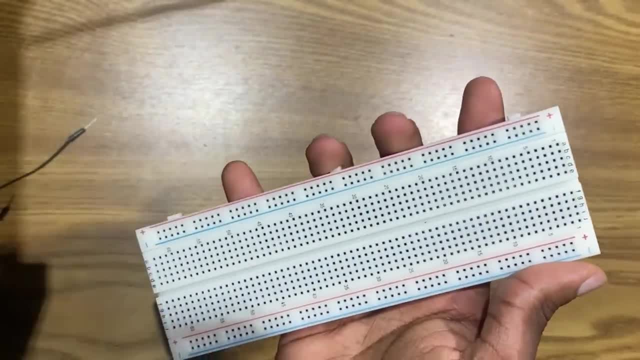 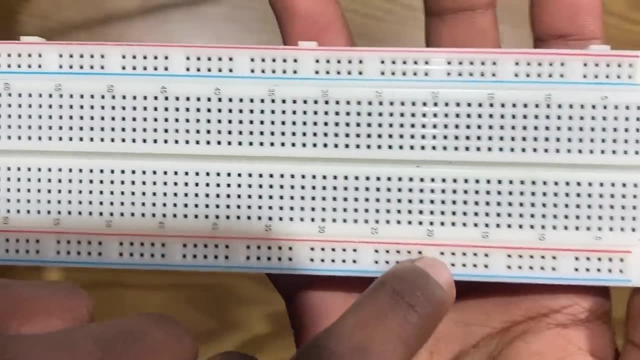 to each other because, as I said again, there is this big gap. Okay, With that in mind, when you look at the ones that are found on the edge, as I said again, if you look at the wires, again, they are connected vertically. So all the way from the bottom to the top they're connected. 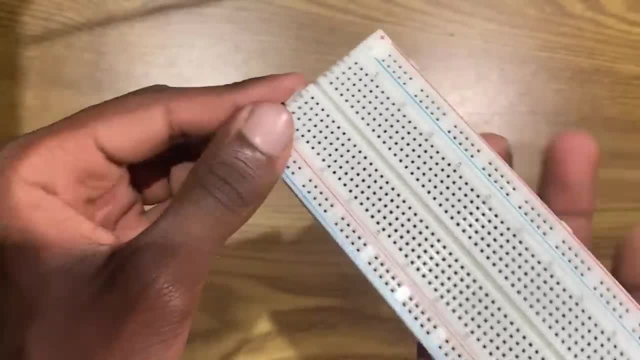 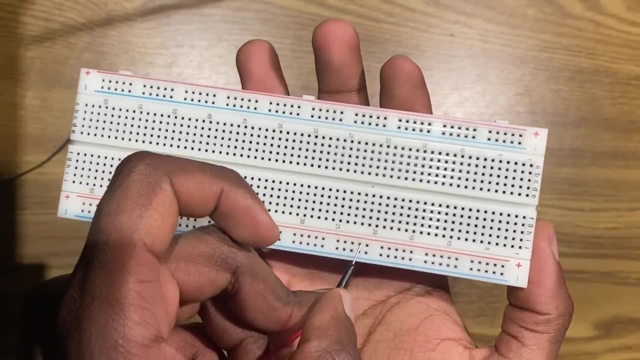 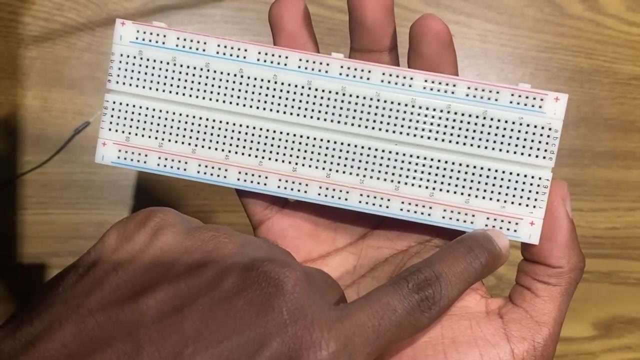 vertically. Okay, From the top to the bottom, they're connected vertically. So it goes like this, So go like this. and you have to go vertically all the way. Okay, All the way. vertically, They're connected. The same goes for the, the one that is found on the most edge, Okay, So. 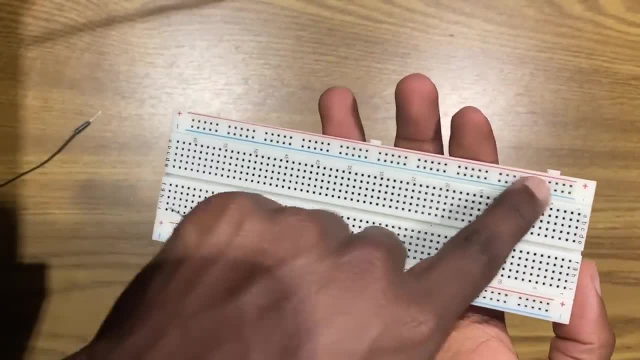 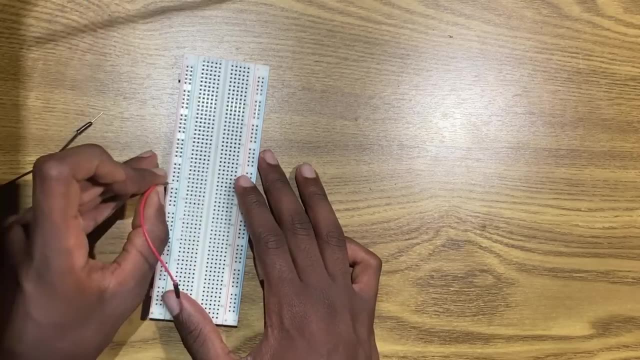 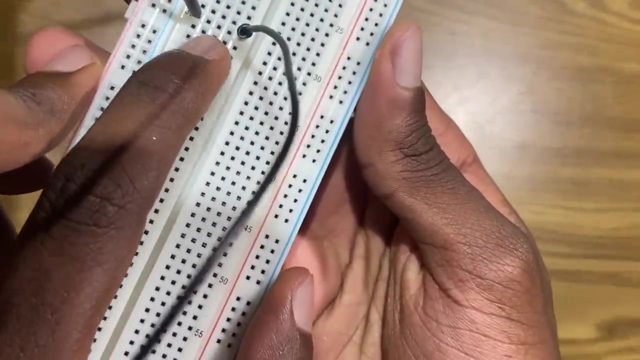 these two that are found on the edge. they're connected vertically all the way. Same goes for these ones. So right now all i have to do to conduct electricity is: uh, bring my conducting wire right here, put that right here and put this right here, and if you again look up close, you're connected because 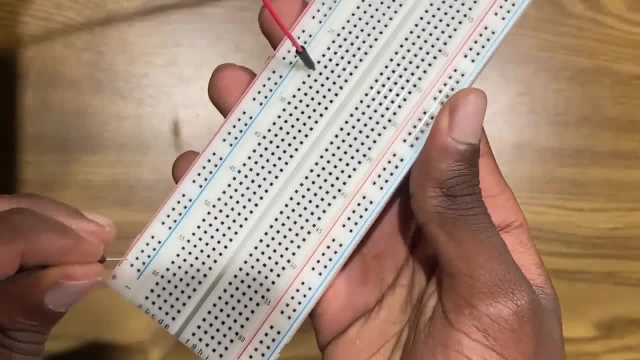 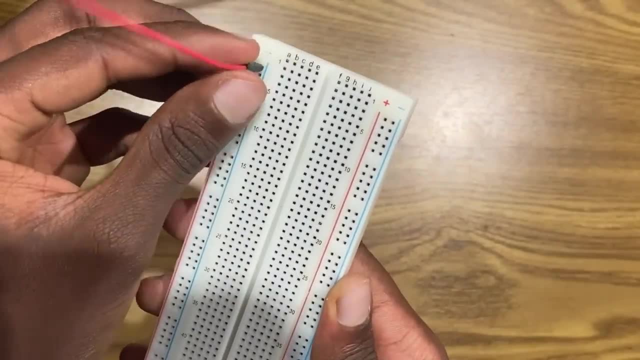 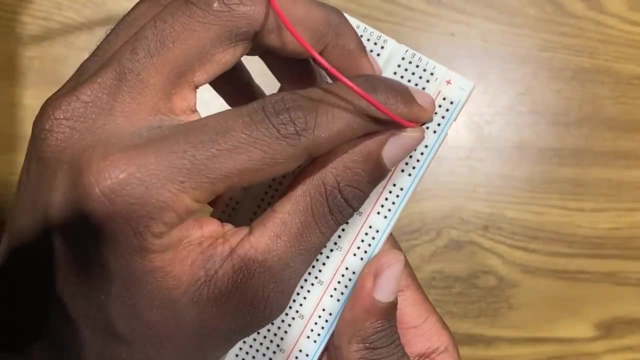 they're in the same row. so if i put this one right here, let's see all the way to the bottom, okay, all the way to the bottom, all the way to the top, oh, okay, they're connected. okay, they're connected. the same goes for these ones too, and these ones and these ones too, okay, so the same. 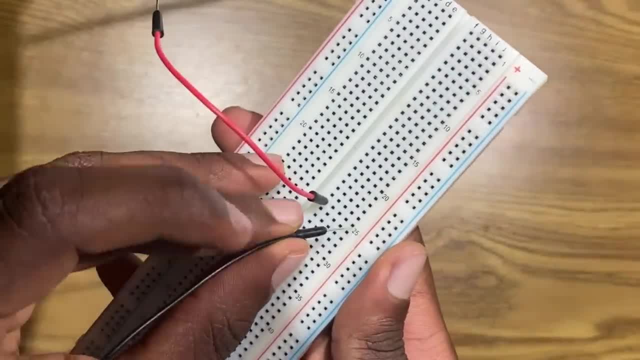 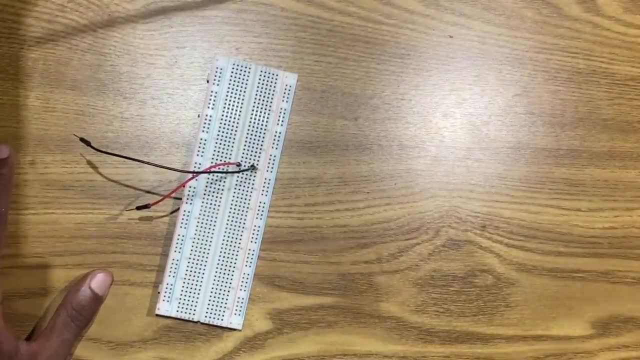 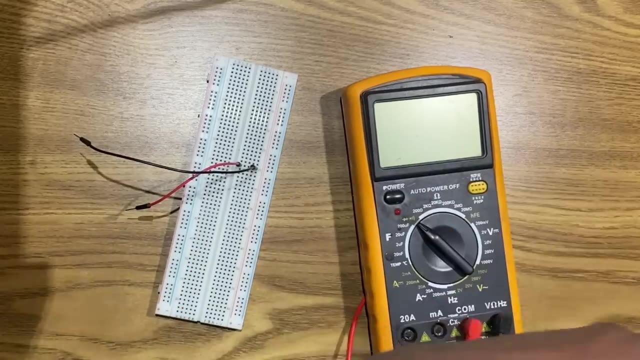 goes for this one. they're connected again horizontally. i just want to recap, okay. so let's say, i want to check this, like scientifically, so i'm going to bring a device called a multimeter- you guys do not need to have it buzz- just again to check, um, okay, so let me just bring that right here. 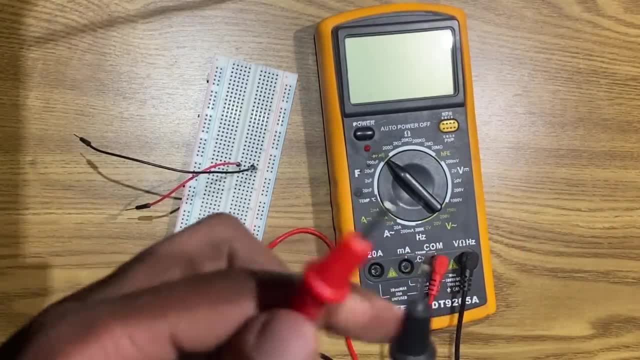 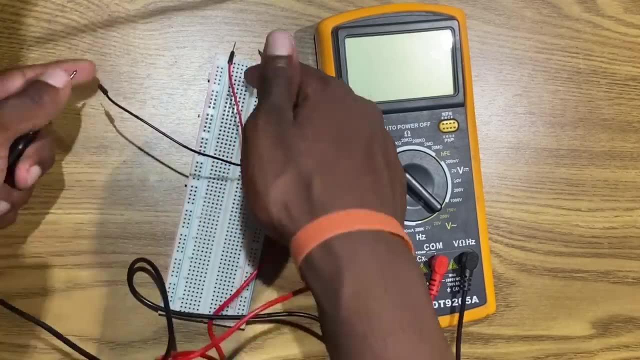 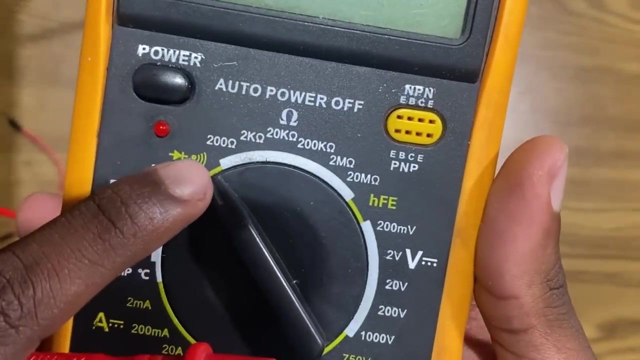 it's a bit tangled right here, okay, so let me just bring this. the pins are big so it won't fit in the holes. so what i'm going to be doing is using this conducting wires and just connecting them with the conducting wires, the pins. okay, so now, if you look up close, it's set in the mode of continuity, okay, this? this basically means this: 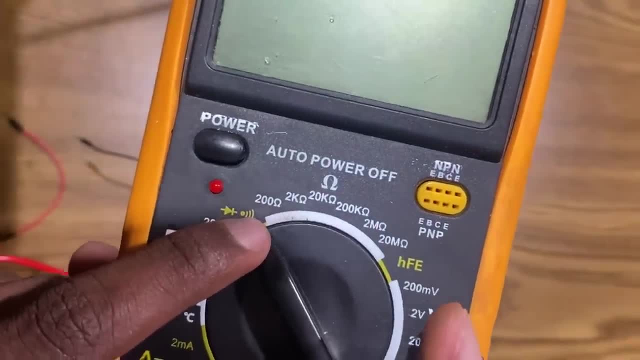 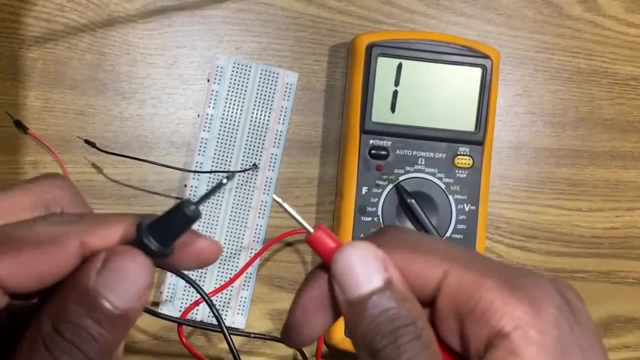 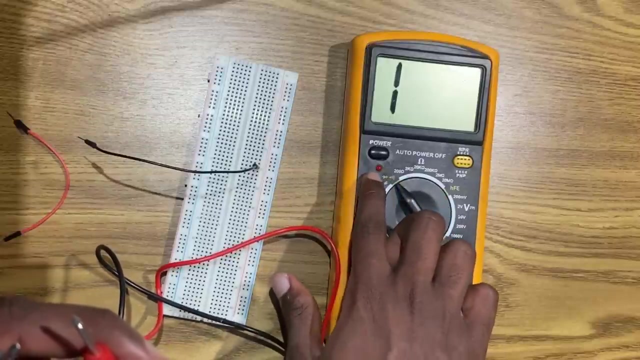 continuity, and continuity checks if an electric current is going. so, for example, let me turn this on. we turn on the power, and if i bring these two pins together, it starts to make this beep sound. and not only that too, but also this red bulb lights up, and so does the number change. okay, 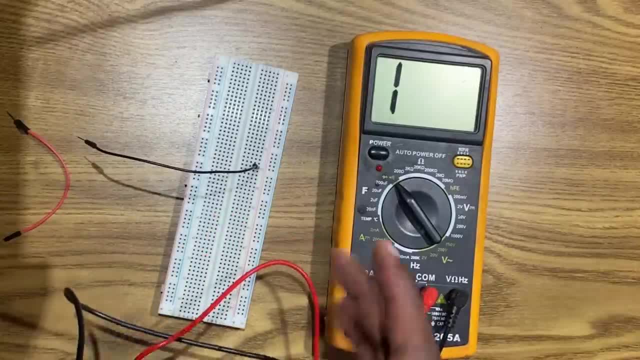 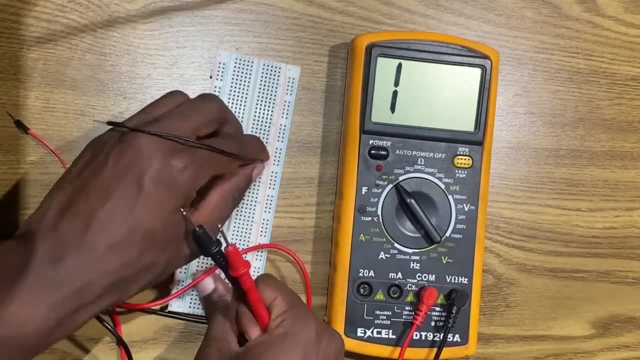 okay. so with that in mind, we can know that there's electrical continuity. as i said again, electrical continuity basically means that current can just flow. okay, so with that in mind, let's say, i bring one right here. let me first go up close and show it to you guys. so let me bring. 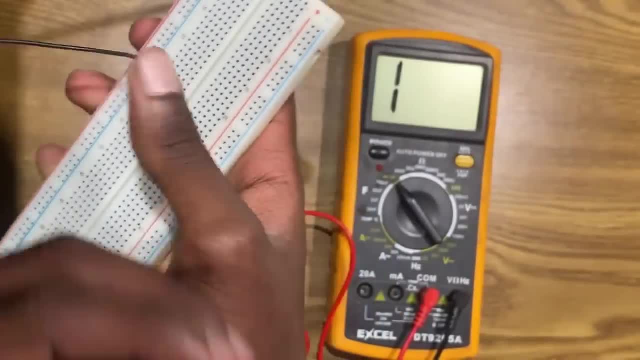 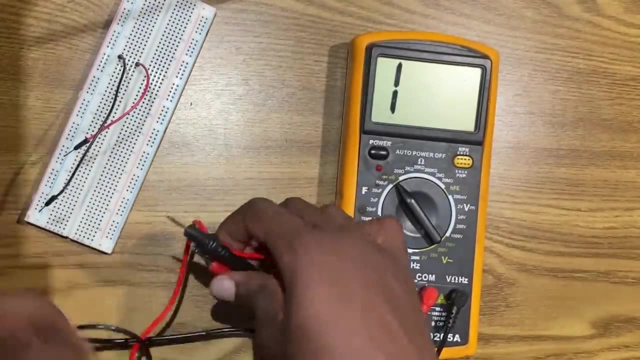 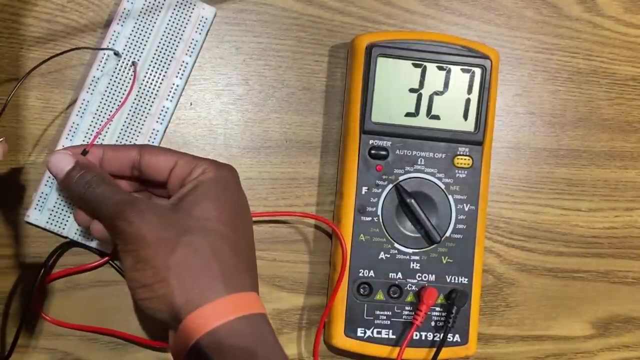 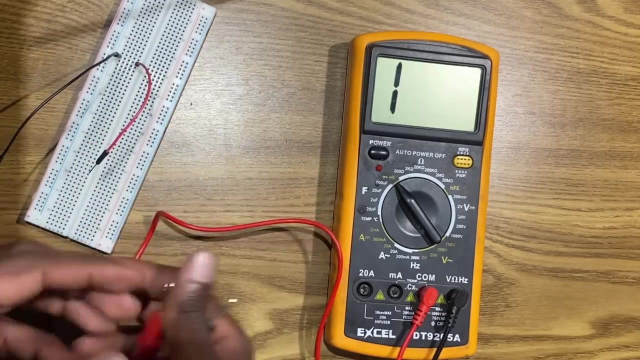 uh, connecting wire to 20 and bring another connecting wire to 20, again connected horizontally, perfectly horizontal. let me just put that right here. and let me bring these two pins and connect them with the wires. can you hear that there is an omnia speak? okay, that means that, hey, it can flow. 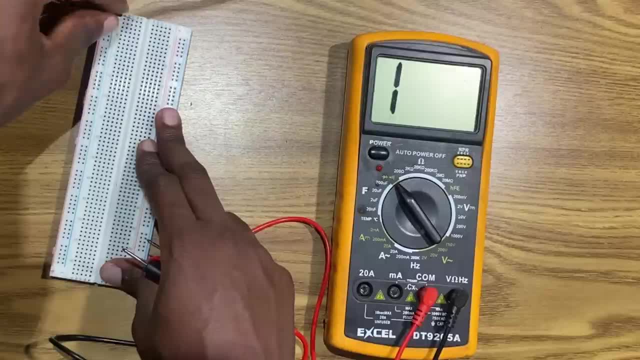 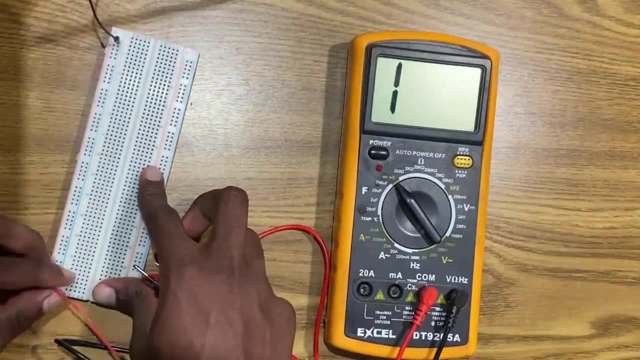 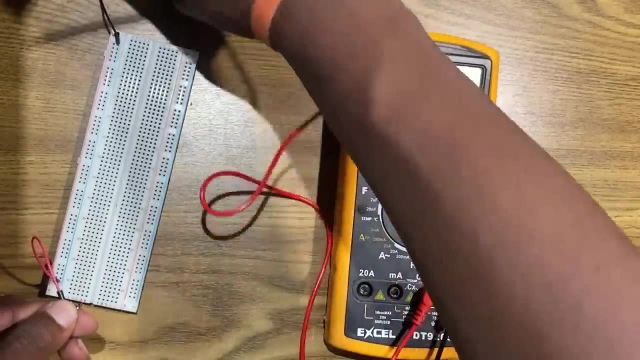 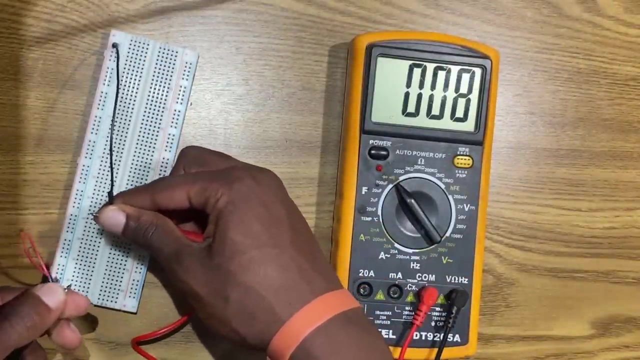 okay, with that in mind, let me just connect this vertically all the way. let me go the whole way. okay, vertically, say i want to connect them. let me just bring this pin right here, right here, let me just bring this to. can you hear it? there we go. this basically means this: hey, a current can just flow through, okay. 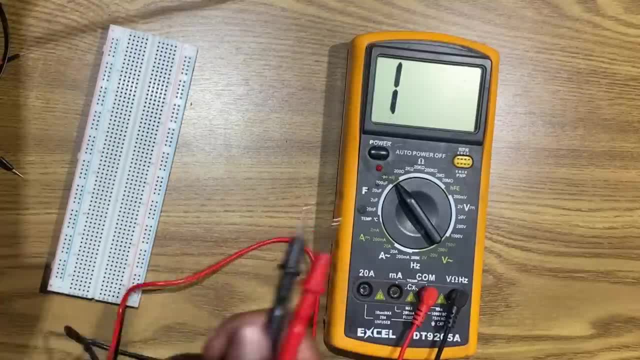 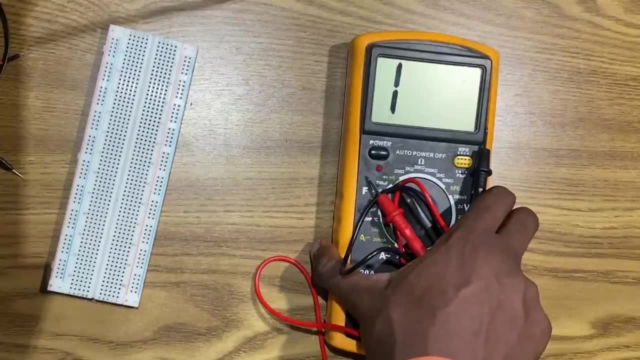 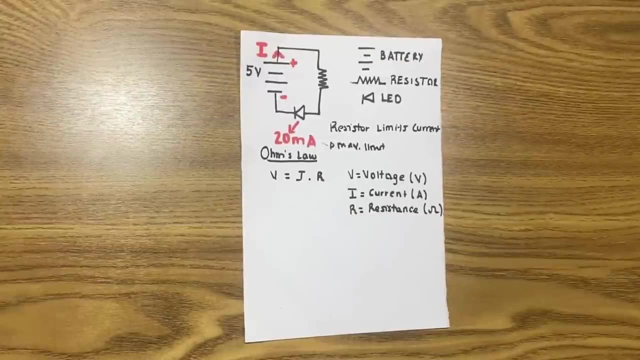 because they're connected right here. they said vertically. so, with that in mind, well, let's move to the next one section where we're actually going to discuss about resistors. so see you in the next one, okay, so in this section we're going to discuss about resistors. so what are resistors? resistors- 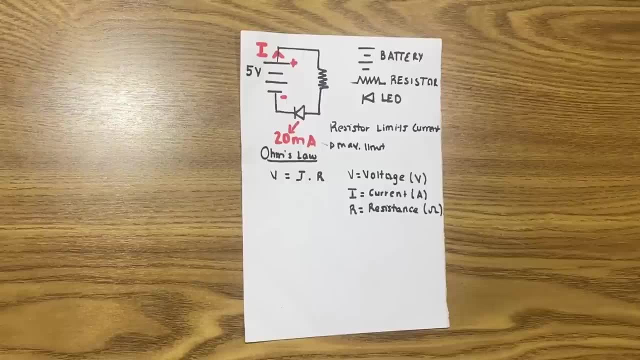 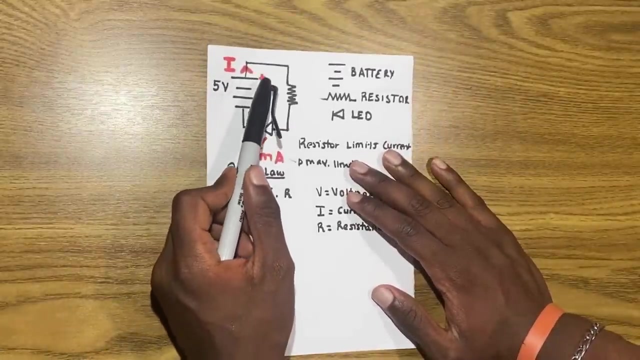 are electrical components that are used to limit current. this is going to be important because we don't want to damage other components due to current overflow. okay, so let's start from this simple diagram. okay, so right here, we've got the positive terminal of the battery. the longer 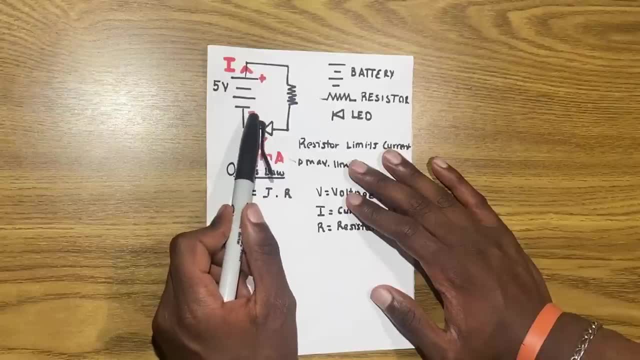 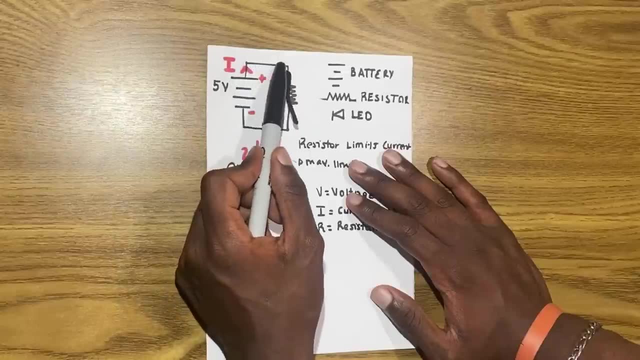 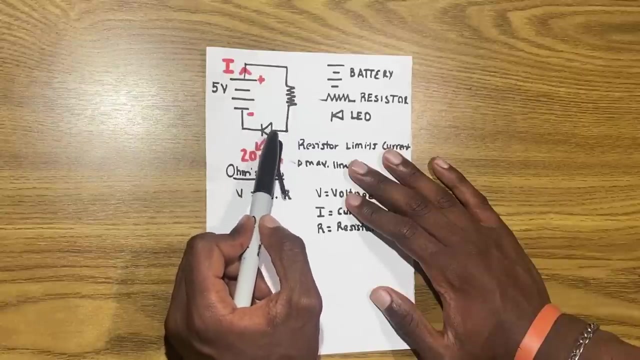 side is the positive terminal, as you can see here, and the shorter side, right here, is the negative terminal. so current always flows from the positive terminal to the negative terminal. so it's going to flow like this: go through this resistance right here and then go through our led lights, up our led. 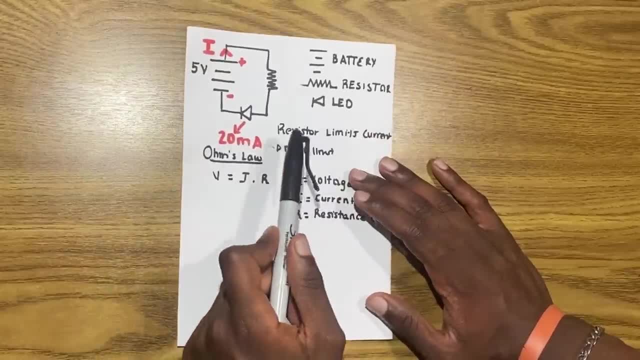 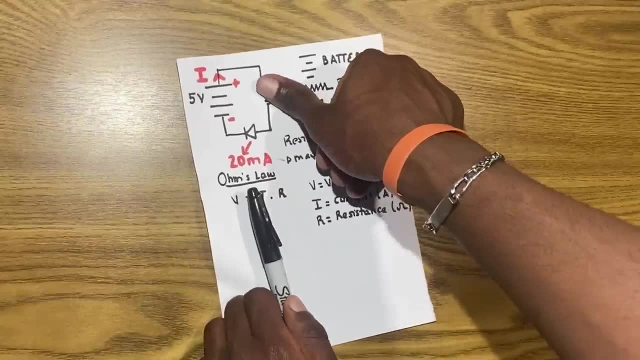 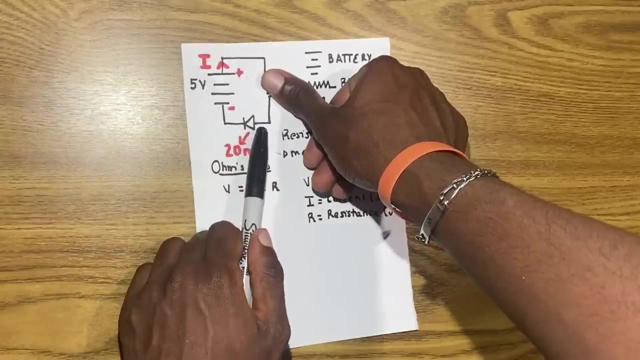 then goes back to the negative terminal. as i said again, resistors are used to limit current. why is this important? so, if we let's say let's forget about the resistance existing here for a moment, so let's say we connect it directly, directly to the current and we put our led- in this case, we're going to fry our led. 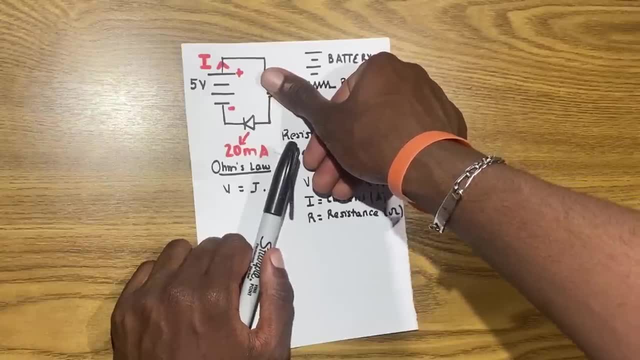 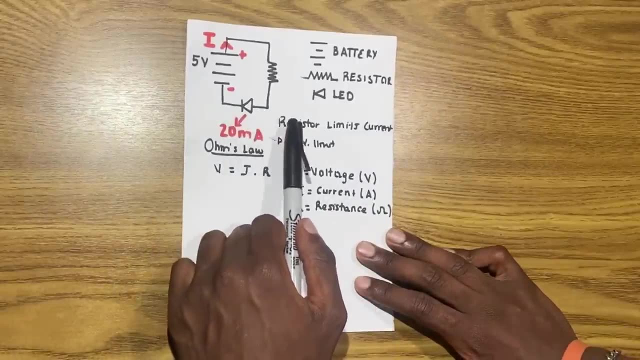 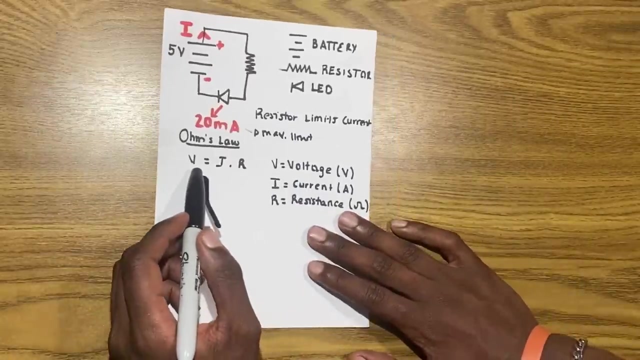 because if we're going to be using too much current, okay, so we want to limit the amount of current that goes through, because we don't want to damage our led. that's why we're going to be using resistors. so right now we're going to use arm slow. it's known as. v is equals to i times. 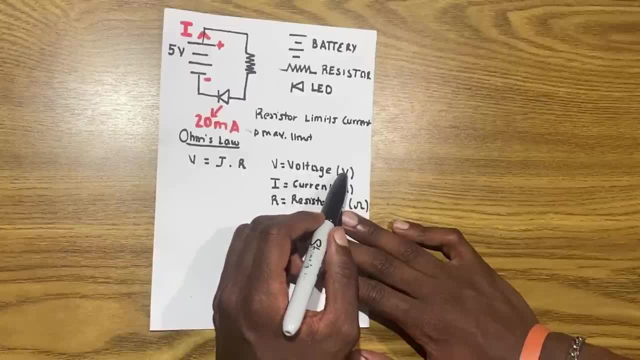 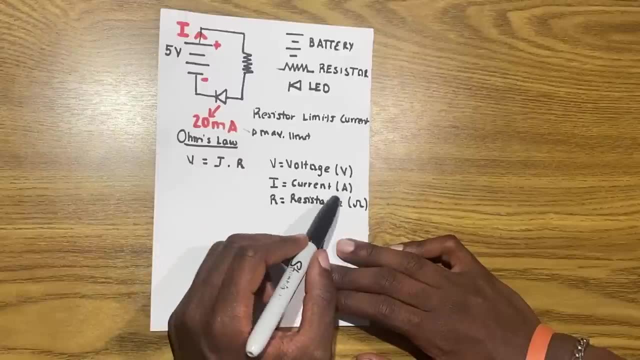 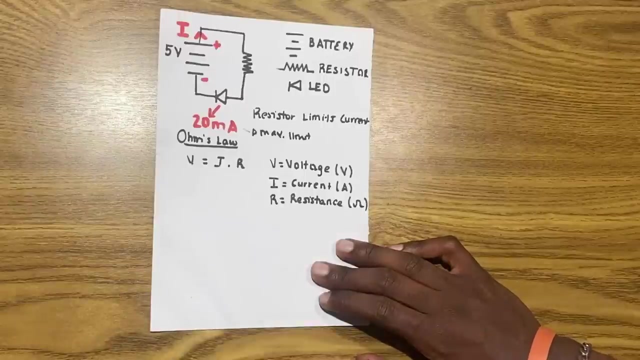 r. v stands for voltage, which is measured in volts, i stands for current, which is measured in amperes, and r stands for resistance, which is measured in ohm. this is ohm, the symbol. you see, right here it's ohm. oh, okay, so right here to actually even give you a better and 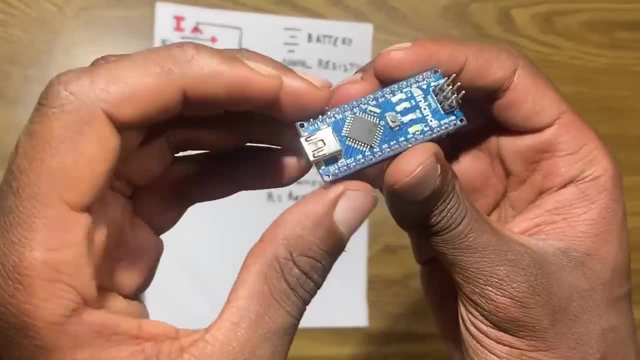 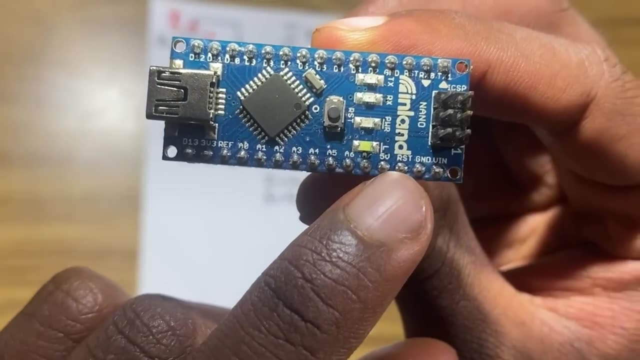 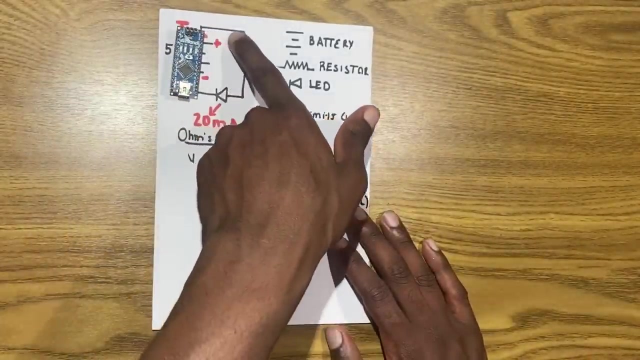 a clear analogy. let me bring my arduino right here and let me bring this close, close enough so that you guys can see the 5v. that 5v means that it's going to output 5 volt. okay, so that's why i said 5 volt right here. so let me just place it right here, then current goes and then we have our. 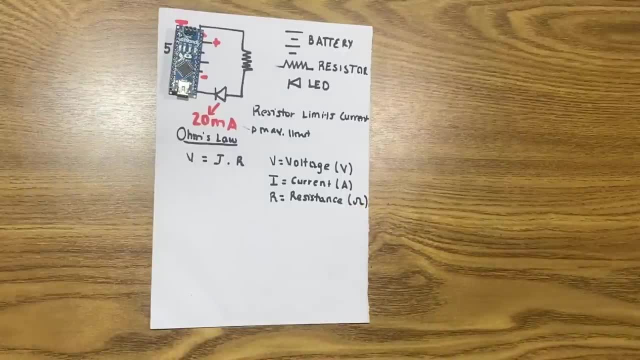 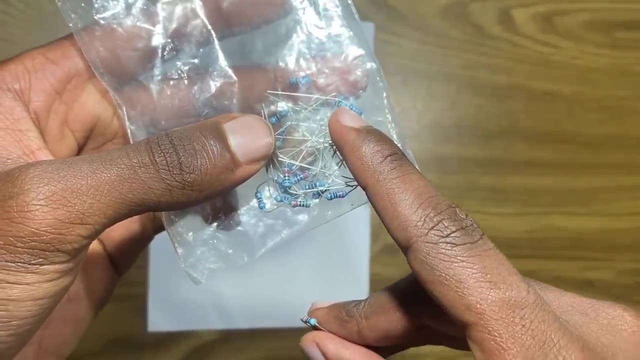 resistor. and, by the way, if you don't know how resistors look like, they look like this: let me bring the pack and let me show it to you guys. they look like this. sometimes you might have find a yellow one, but it's okay. blue or yellow is the same thing. okay, so we have our resistance. 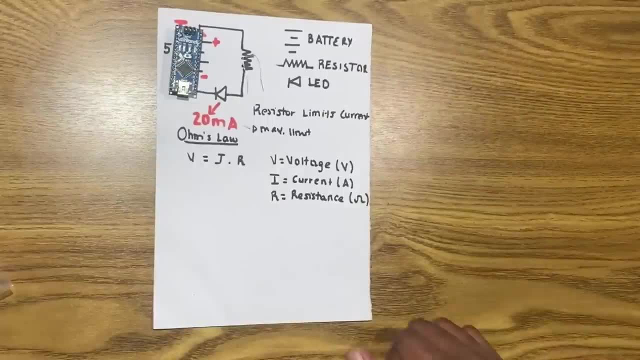 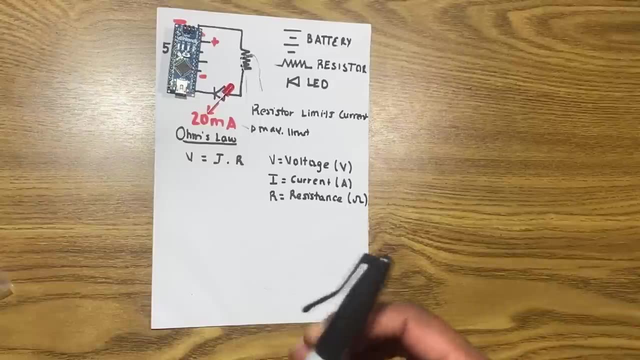 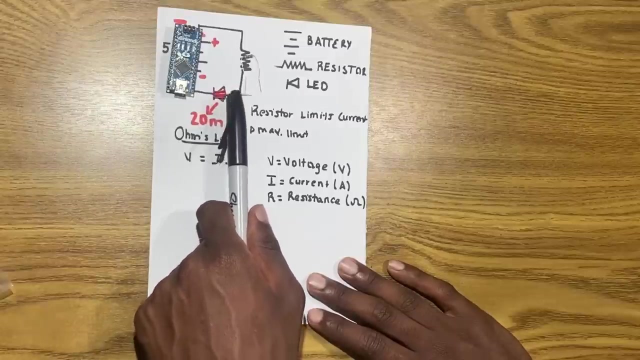 right here. let me place that right here. and we have our precious led. let me just place that right here. so right here. when it comes to leds, they have a maximum limit of 20 milliamps. so if we go over 20 milliamps, what's going to basically happen is we're going to fry our led. 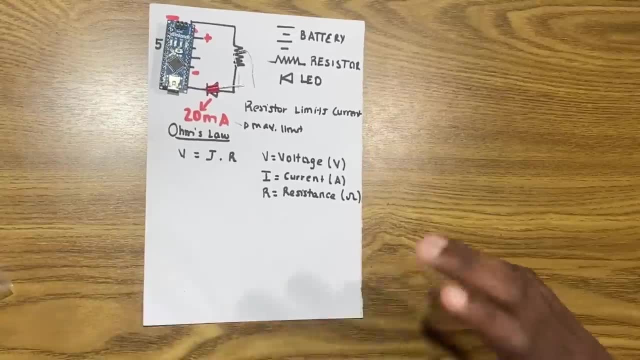 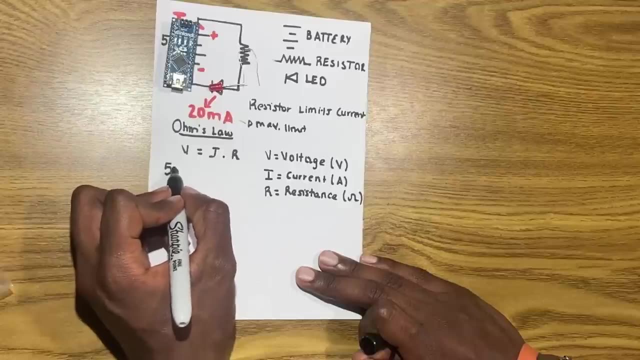 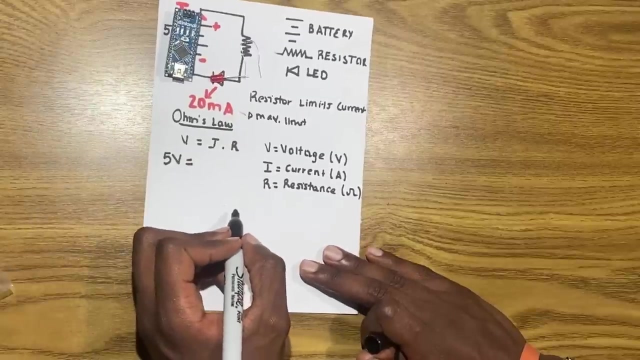 so we don't want that to happen. how do we prevent it? we use this level. so right here we have 5 volt that is going to be output by the arduino. so we're going to say 5 v, say calls to this is 20 milliamps, is the maximum. the recommended one is 10 to 15 milliamps. okay. 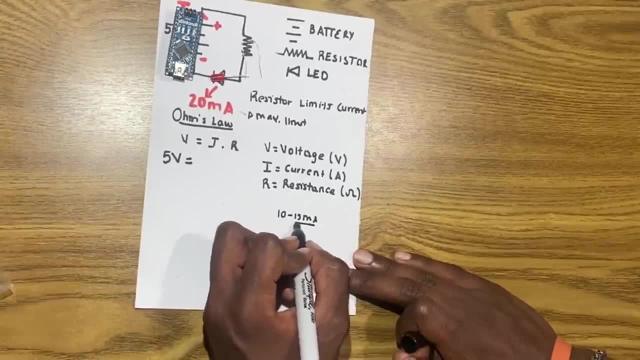 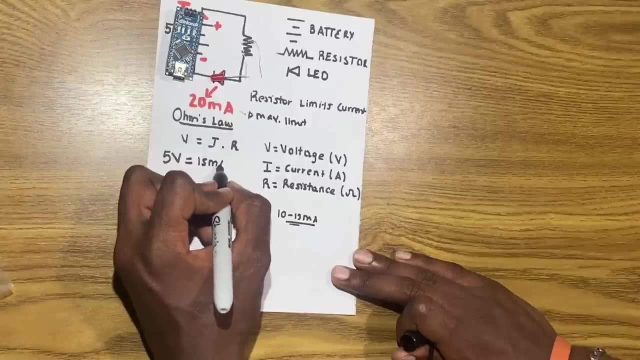 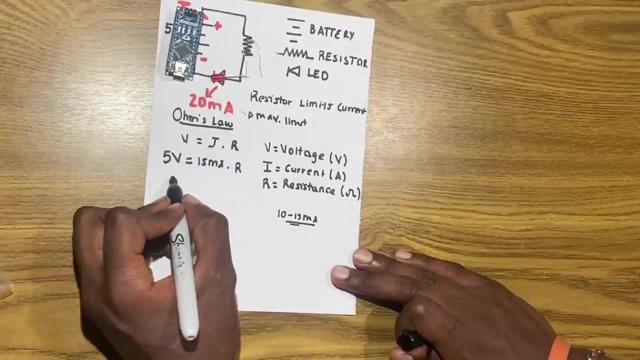 it's 10 to 15 milliamps is recommended, but this is like the. this is like the full maximum, so let's use 15 milliamps because we don't want to go over the recommended limit. we have our resistor right here. okay, so let's divide this. this becomes 5 or 15. 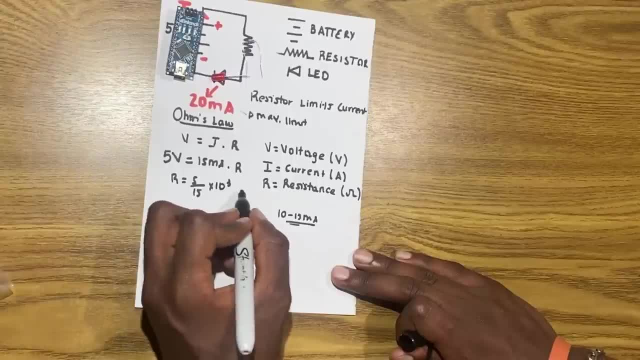 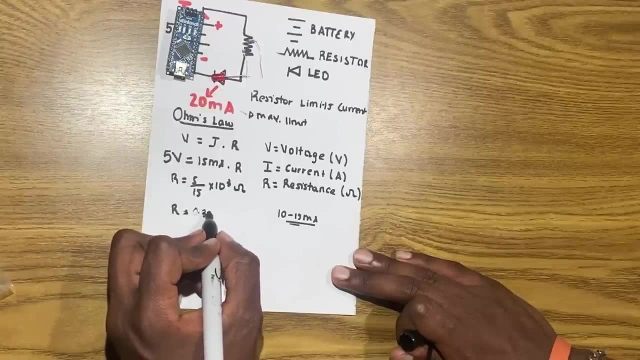 and we have milli right here, so it's going to be times 10 to the power of 3.. we've got our ohm. i said earlier it's measured in ohm, so in this case it's going to be 0.3, continuous. 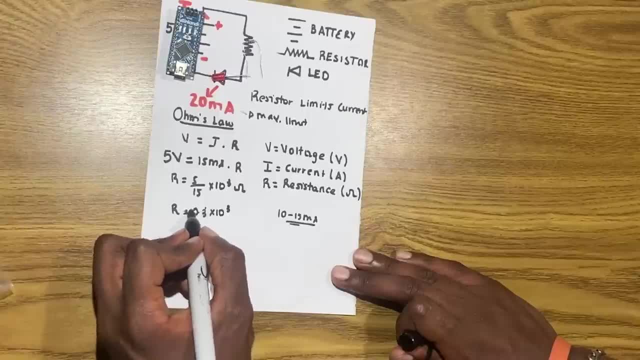 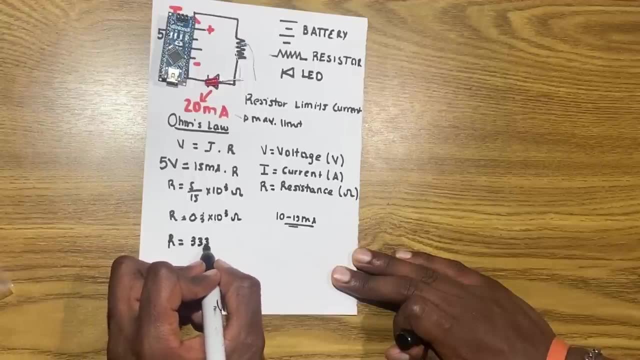 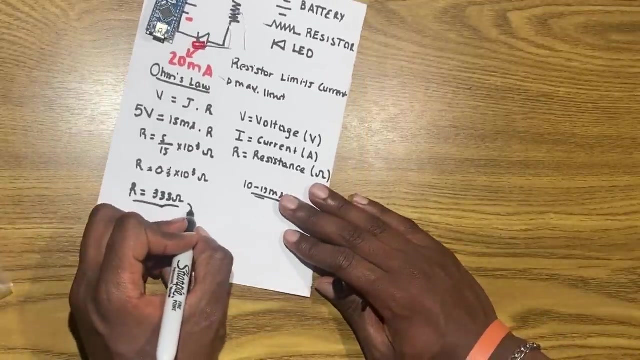 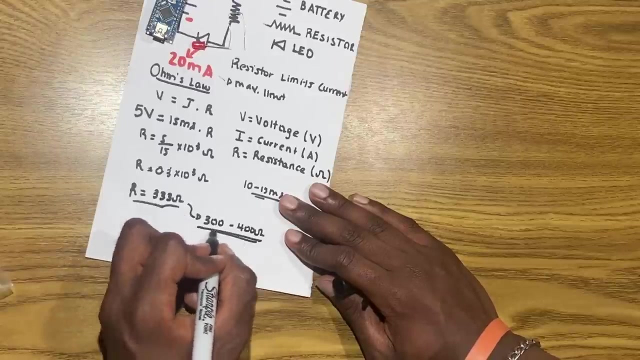 times 10 to the power of 3. okay ohm. so r is going to basically be 300 and 0.33 ohms. this does not mean we have to exactly give it 333 ohms, or rather we should give it a range of, let's say, 300 to a 400 ohm range. okay, of resistance for this current, not to obviously. 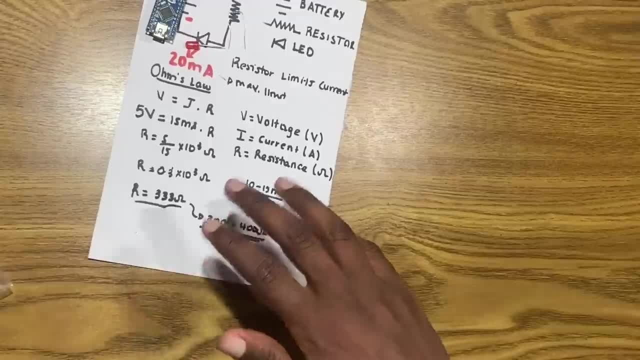 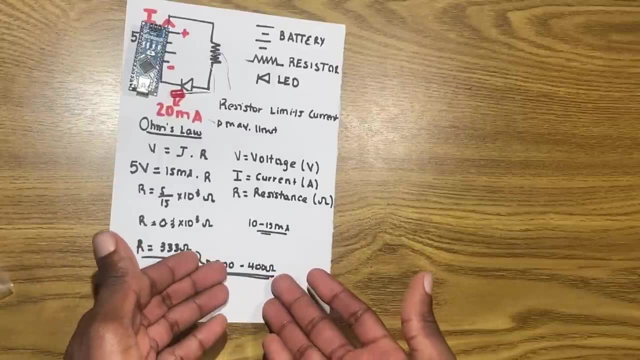 overflow and, as i said again, basically fire led. we don't want that again to happen, okay. so, with that in mind, how do we, you know, measure how much ohm resistance is? so we're going to actually check it. so let me bring. there are two ways to actually. 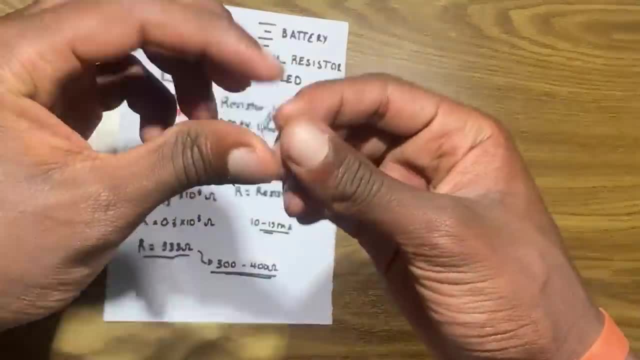 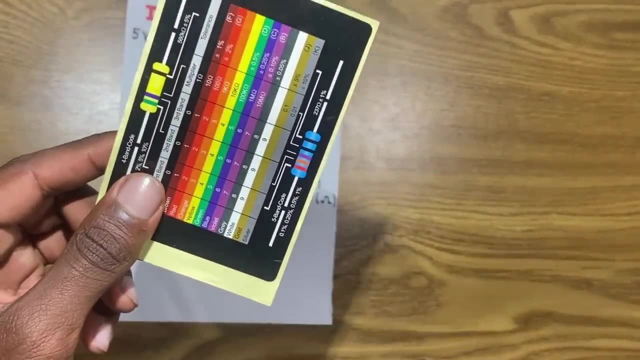 do it? the first one is we bring our resistor up close. okay, and what you need is a resistor color code. you can google it if you don't have it on your kit or you don't have an arduino, but this is just a resistor color code. so right here, i have it. right here. 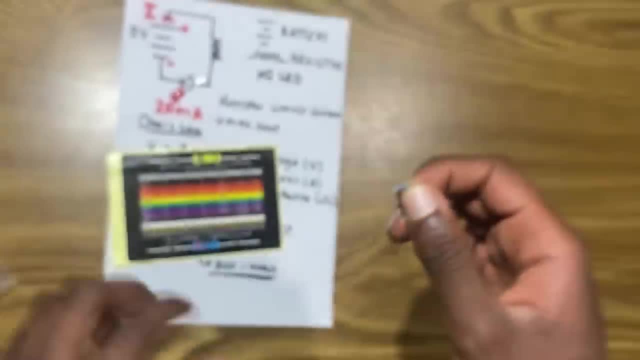 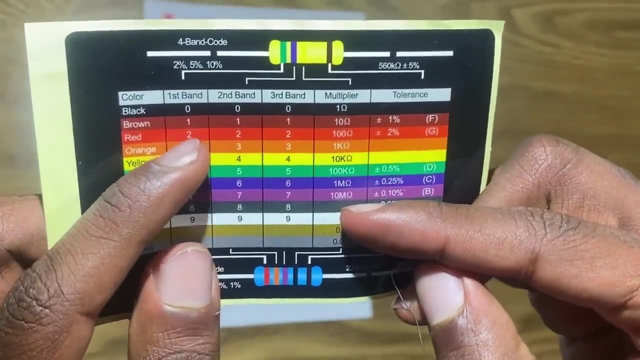 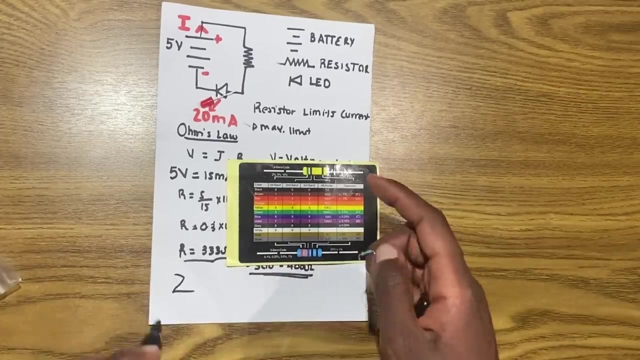 so let me start from the first line. the first line is red and if you look close enough right here, first line of red means two. so let me bring my sharpie right here, let me write two down. you got two. now let's look my. let's look at my second band right here. 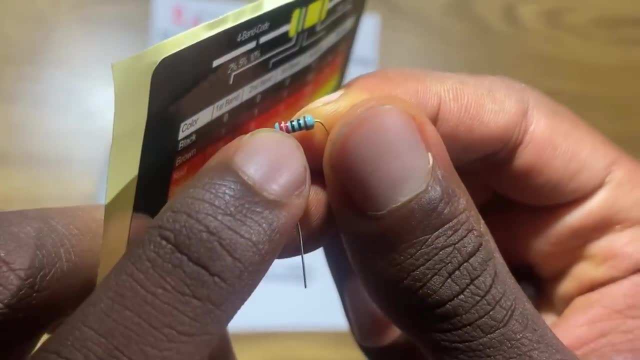 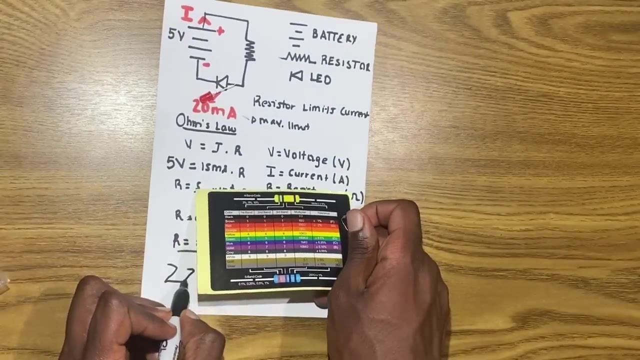 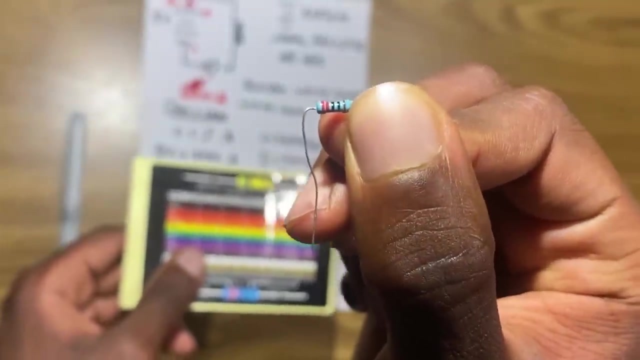 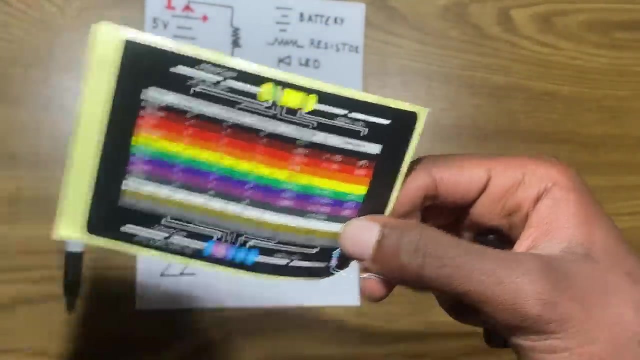 it's also red. you can see it, it's also red. second band of red means two. so we go two right here. then i have my third one. you can see closely, it's black. so when we look at it right here, when you look at the third one, it's what? it's zero. 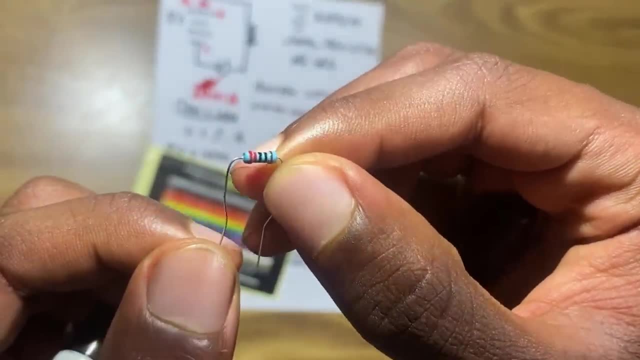 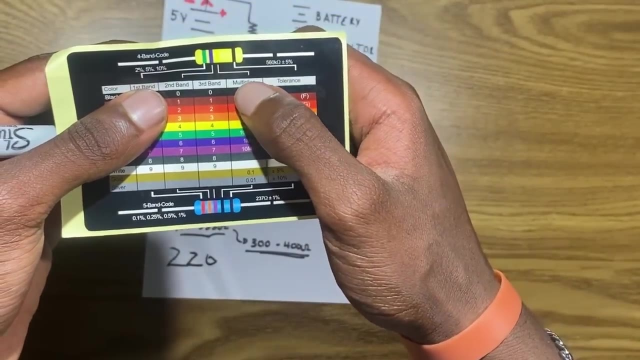 okay, then we have my fourth line. my fourth line is also black, so i go to the fourth one and it's a multiplier. so this is basically how much i multiplied two. so in this case it's black, so it's times one. and then i have my fourth line, which is also black, so i go to the fourth one and it's a multiplier. so this is basically how much i multiplied two. so in this case it's black, so it's times. 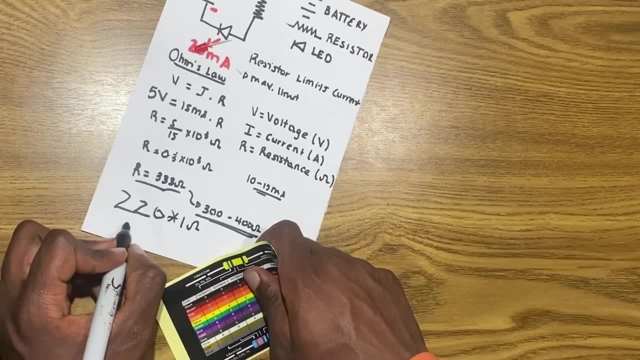 one. and then i have my fourth line, which is also black. so i go to the fourth one and it's a multiplier. so this is basically how much i multiplied two. so in this case it's black, so it's times one arm. okay, so when you multiply it, it's 220. 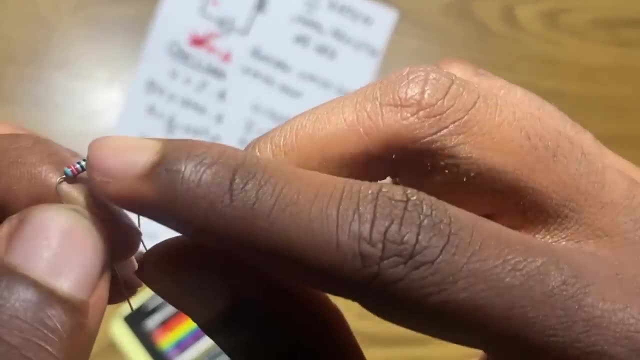 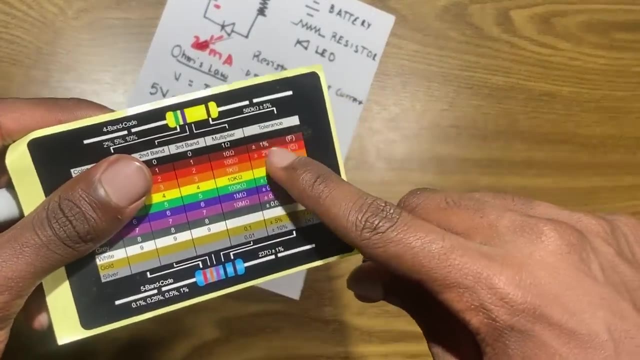 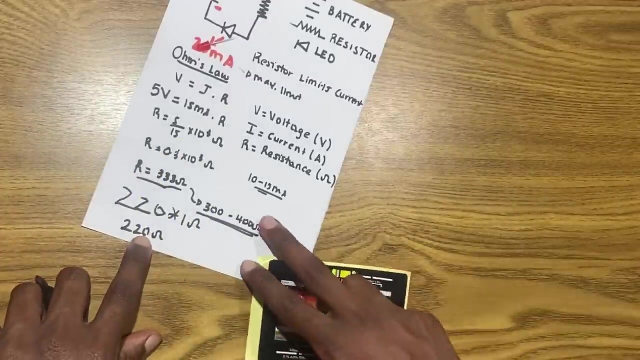 arms. if you look even close enough, there's a fifth band right here that looks brown. this is just tolerance and we're not going to get into it because it's not really important surrounding this level. okay, so okay. with that in mind, we have 220 arms of resistance. 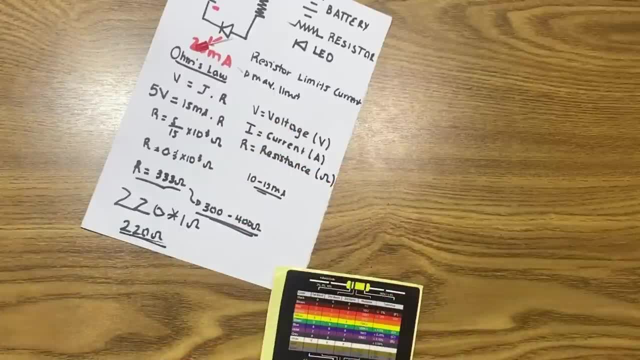 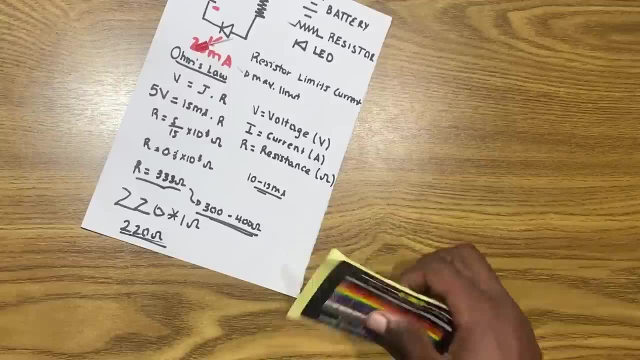 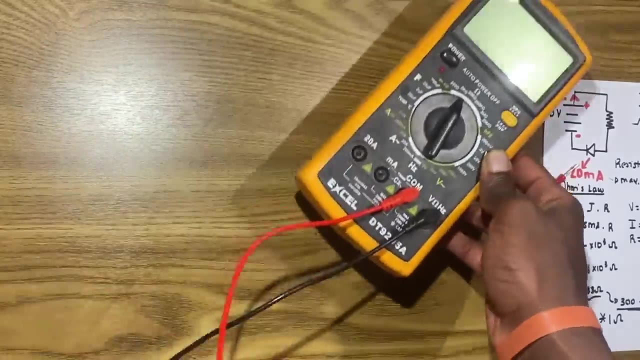 so you guys can check your resistor by basically looking at the color codes. okay, there's also another way to actually do this. so in this case we're gonna go back to using multimeters. so right here we have our handy multimeter. let me just untangle it right now. 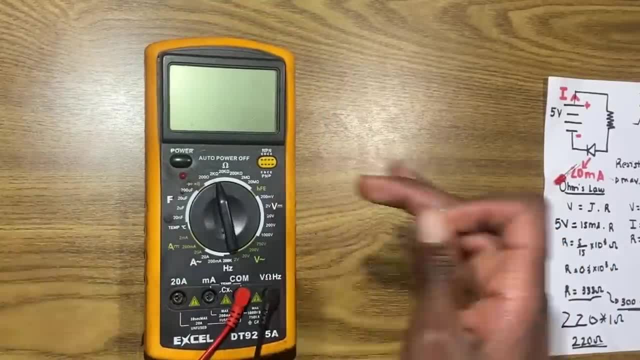 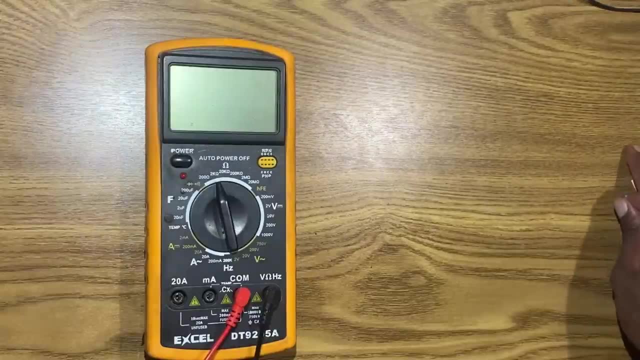 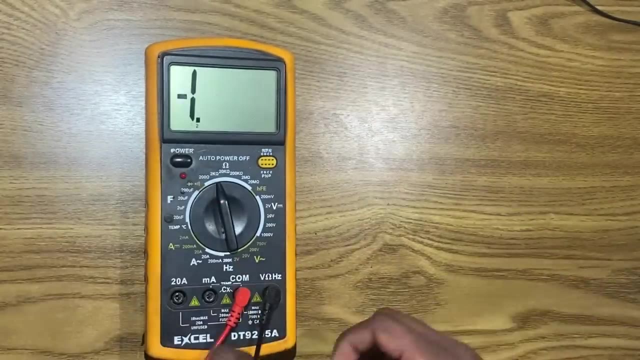 okay, so let me bring back the resistor that i had here, that i calculated to be 220, right here. so let's see if that's actually true. if i want to be dead sure, okay, so let me just move this paper right here. okay, so let me turn it on and right here, what i'm going to basically do is change it to the resistor mode. 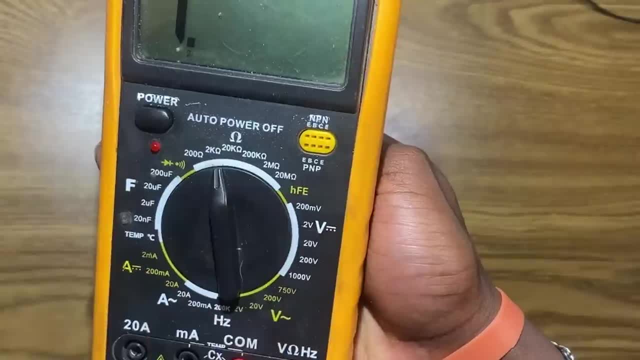 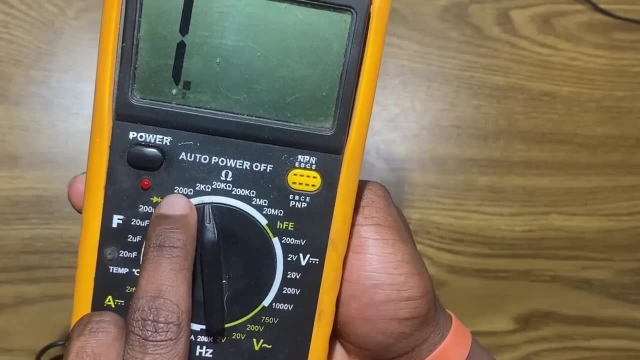 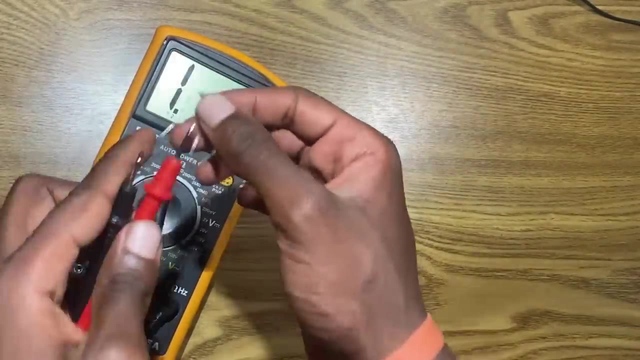 as you can see, there's arm right here. so we're changing into this resistor mode. so if i go to 200 ohm right here, it's going to detect a one. it's going to detect 200 ohm or less. for example, right now i have 220 arms. that i calculated. if i put it right here, if i again 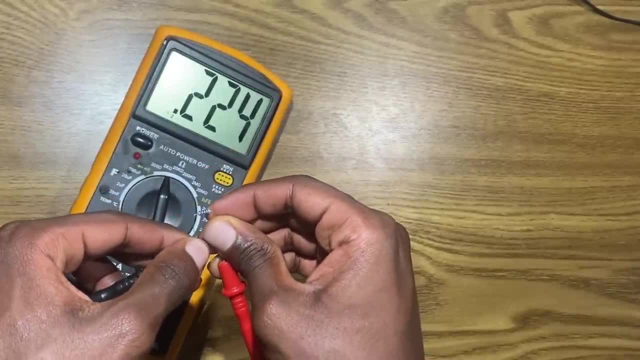 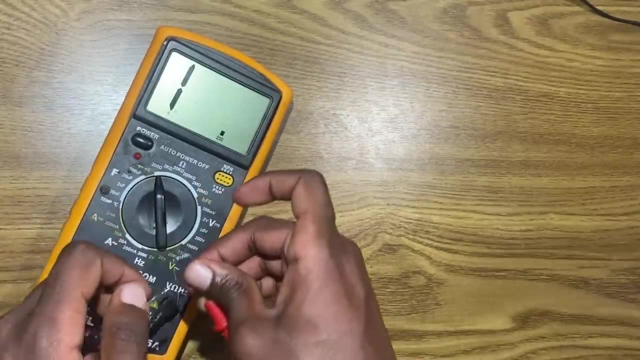 connect it right here. let me just connect it and you guys see it. it says a 0.222. let me change it to 200 arms right here. if i go 200 arms, it's not going to detect anything, as you guys can see. why is that so, you might be asking me. well, it detects. 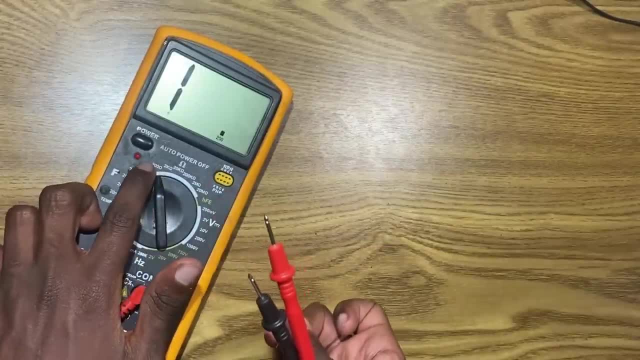 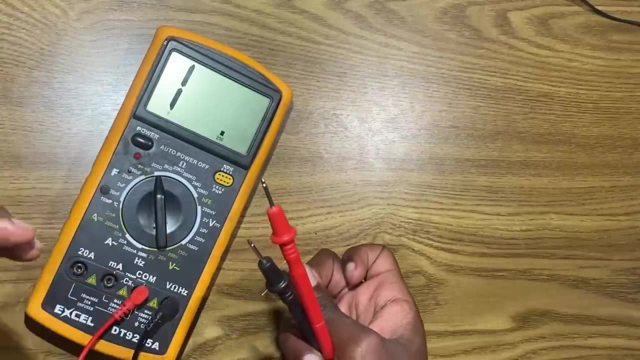 200 arms or less. okay, it's not going to detect 200 um that are above 200 arms. it's going to detect 200 arms and less. it's not going to detect something that is above 200 arms. in this case, this is 220 amps, which is above 200 amps, so we're going to go ahead and change that to 220. 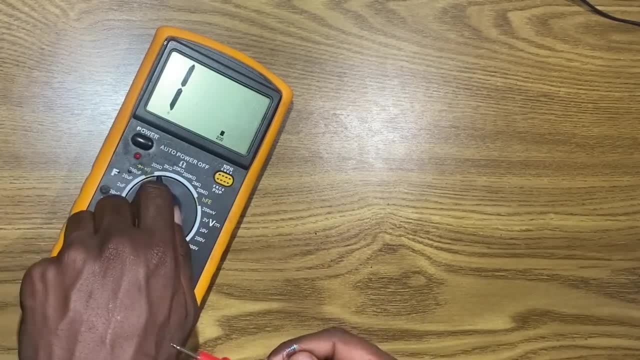 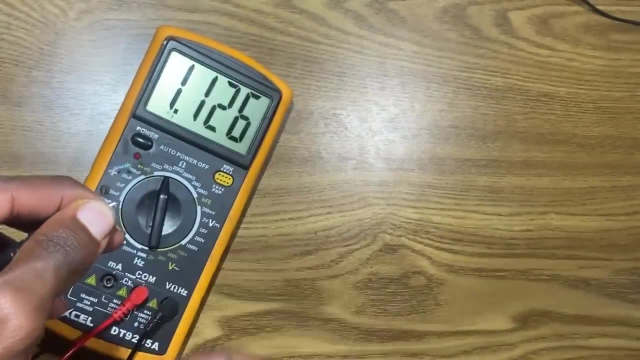 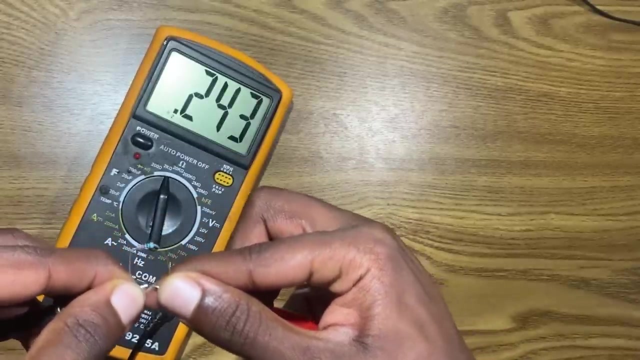 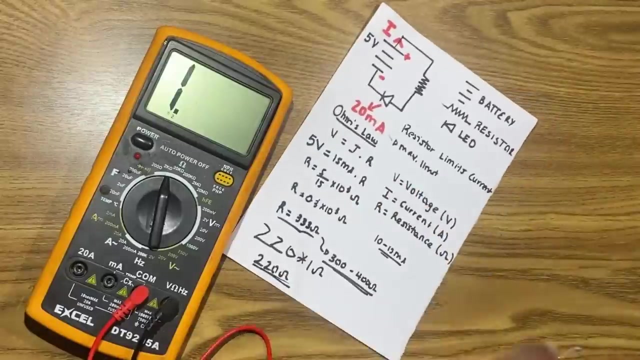 ohms, so it will not detect it. so if i go to two kilo ohms, okay, two kilo ohms right here, and let me just connect it right here now- we get a signal of 2.242, not exactly, but we get 0.242. let me just bring my paper back. okay, so two or two, point two. 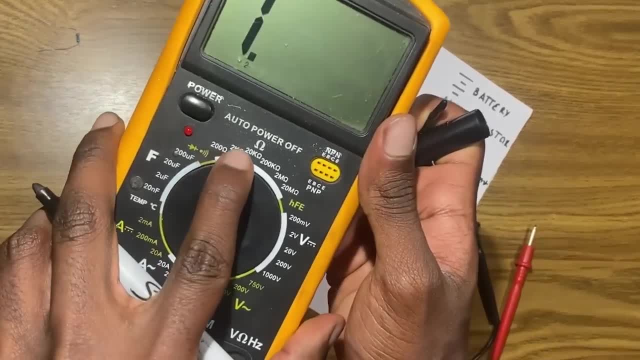 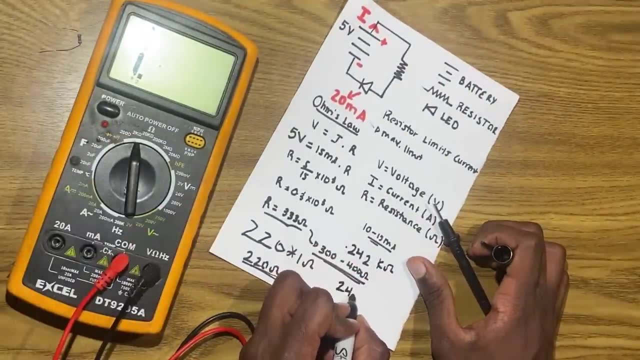 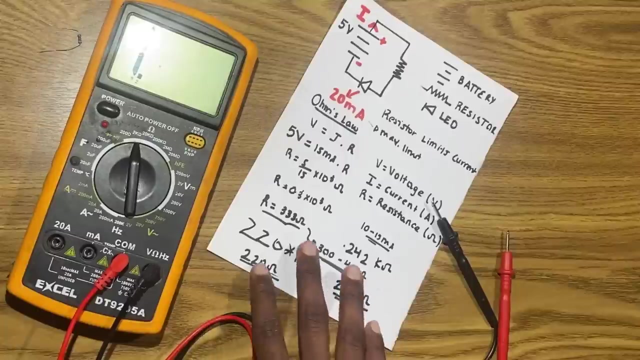 and, as you can see here, it says kilo, so we have to say kilo arms. when we draw it out as a matt, this turns out to be 242, which obviously is not 220 ohms directly, but it's just very close to it so we can use our multimeter. 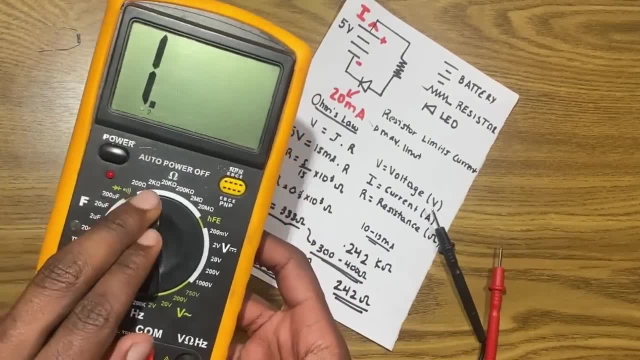 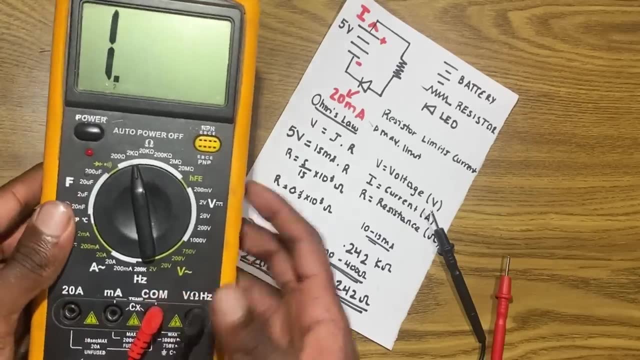 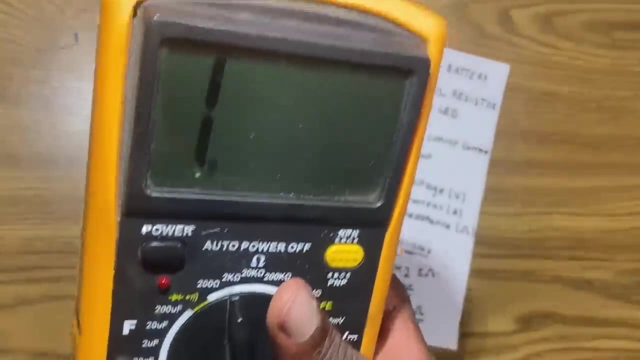 to again check resistance values. it's not going to give you the exact one, but it's going to give you a close one. so you can see. you can see that that is 222. there we go, article 20 ohms going up. use a resistor, resistor color codes right here, or again you can use your multimeter. 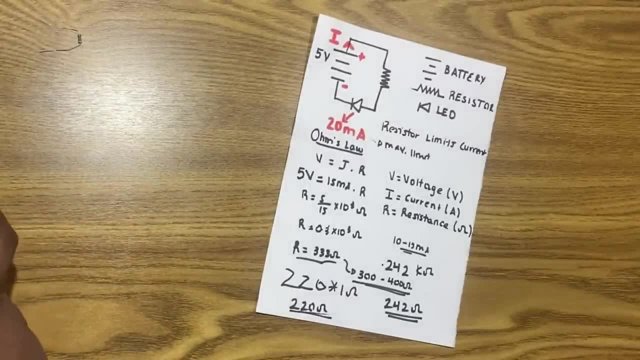 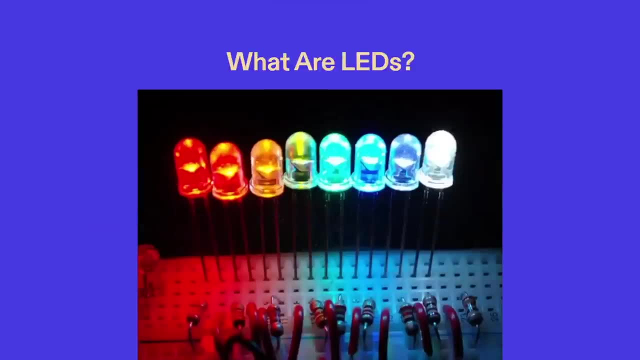 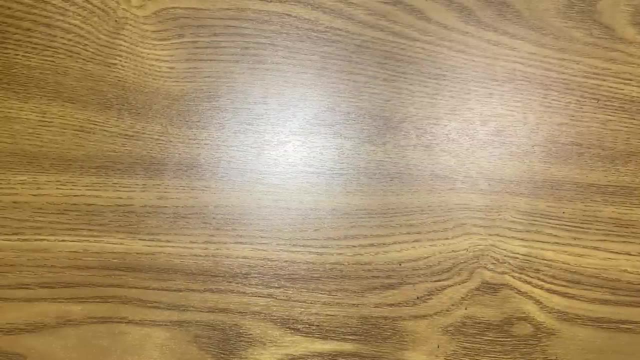 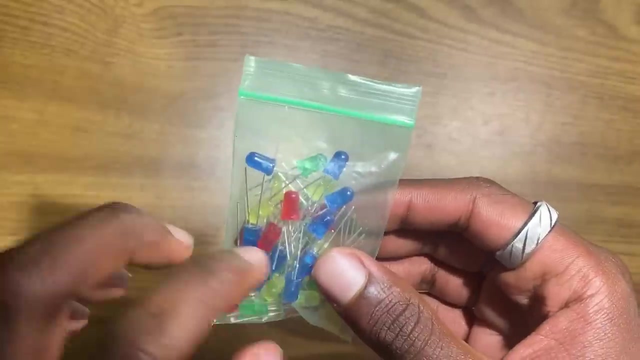 it's up to you to decide. anyways, see you in the next section where we're going to be discussing about leds. in this section, we're going to discuss the last component that we're going to need to build our first project. they're going to be leds. so if you open your pack, 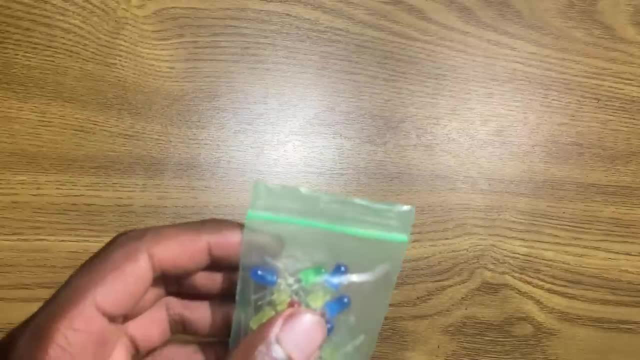 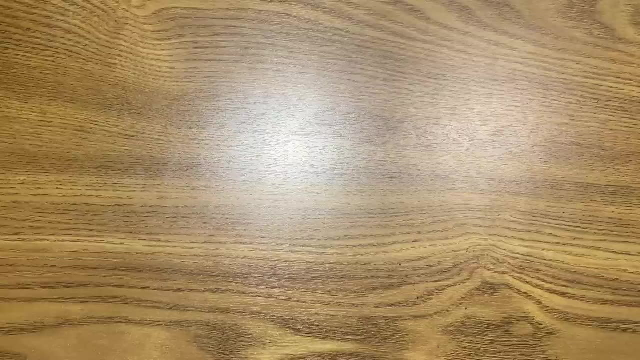 they come in this shape and they come in all sorts of colors. right here we have red, green, yellow. so before actually working with leds and putting them in our project and working with them in the circuit, we're going to basically do is we're going to check the signs behind them. 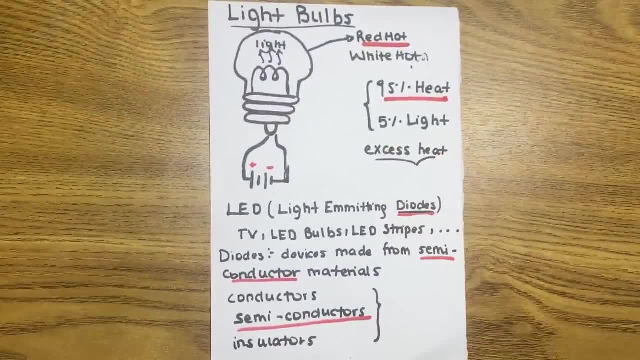 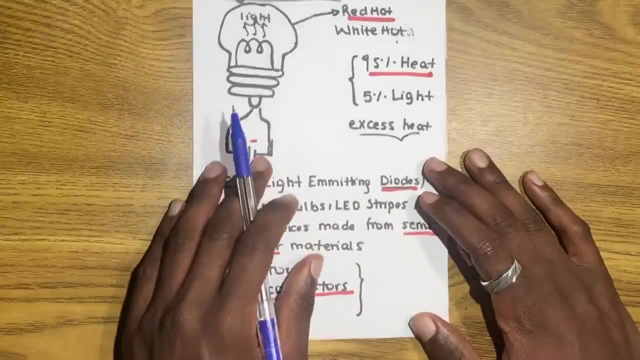 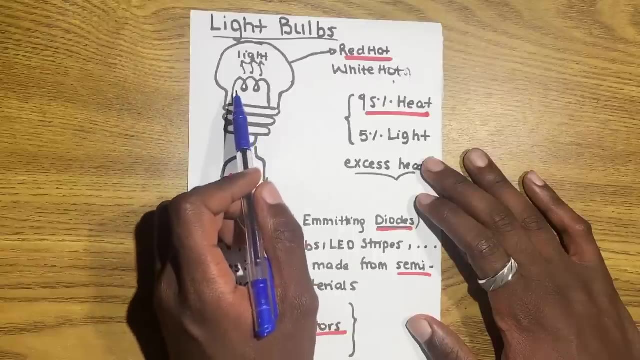 and have a brief understanding of how they work. okay, so let me begin right here with something quite more popular. so light bulbs. light bulbs were obviously invented by thomas edison and let's see how they work. okay, so, right here, we have a battery, right here and it. 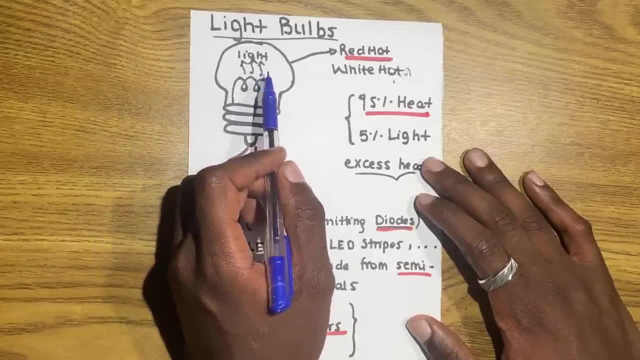 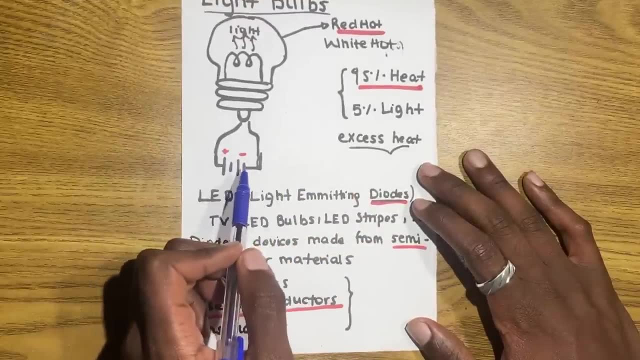 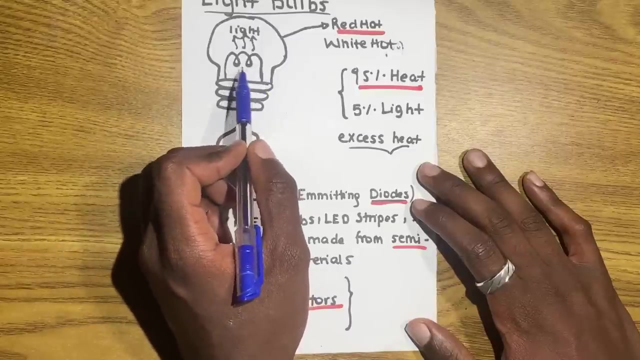 supplies current. so what basically happens is current goes through this coil and it heats it up so much so that it starts emitting light. in this case it is red hot. when we add more wall to this battery or a higher voltage battery right here that we're using, we're going to supply more current, basically making this coil heat more. 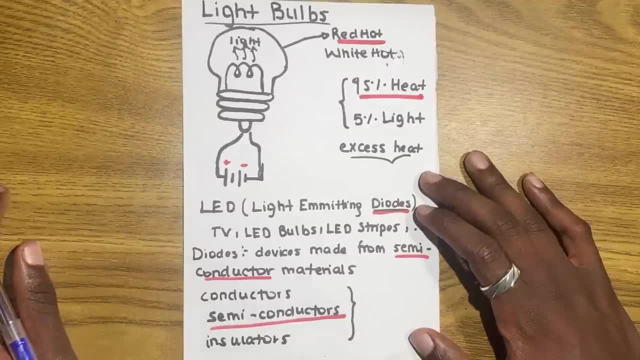 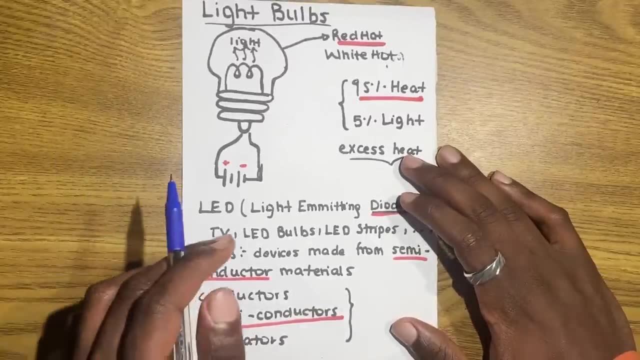 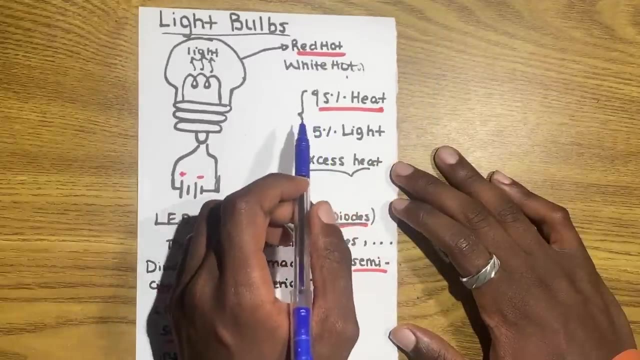 and it will obviously going to emit more light. So in this case, it becomes white hot. So what is the problem with light bulbs and why did we even need to replace them? Well, the problem is, fundamentally speaking. light bulbs are not light generating devices. They are heat generating. 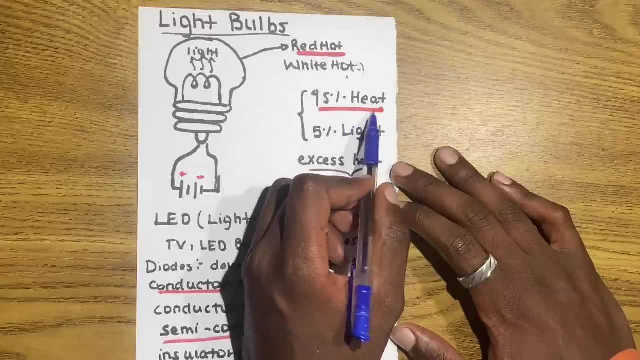 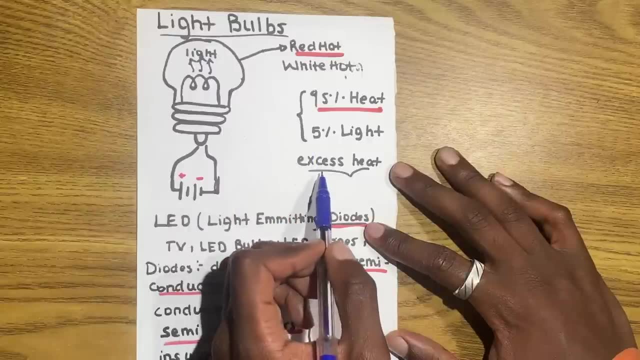 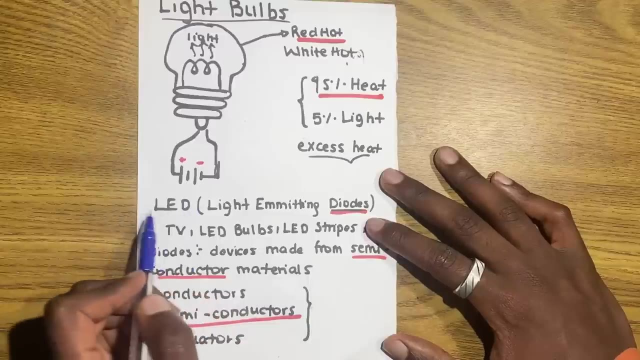 devices, because the electrical energy that we're going to input, the current- is going to go towards heat. 95% of it is going to go towards heat, while only 5% of it goes towards light. So in this case, we're going to be producing excess heat and we're going to be wasting energy. 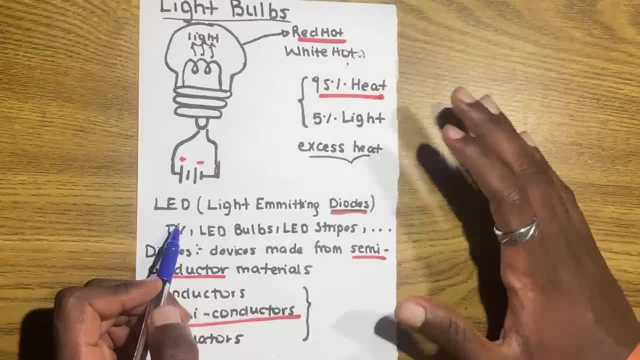 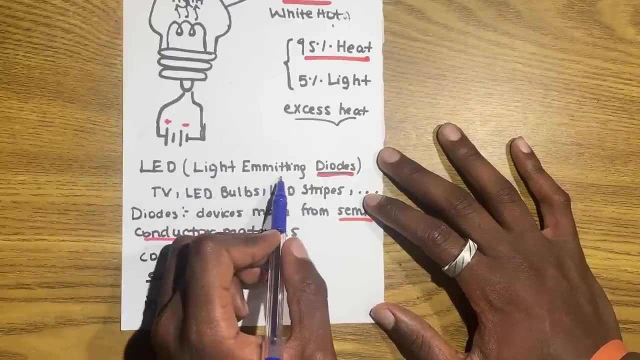 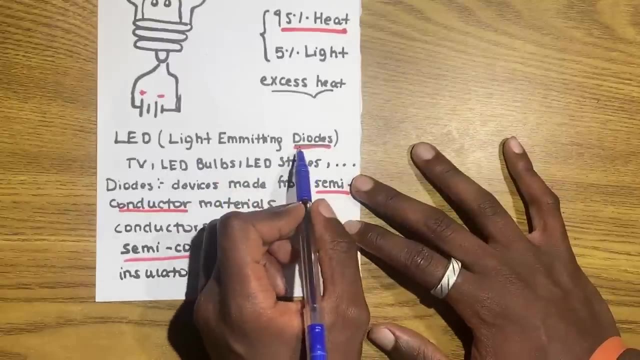 So we don't want that to happen. That's why we have LEDs. LEDs change electrical energy directly to light energy. Okay, so LED, the long form is light emitting diodes. Light emitting is self-explanatory, as it just says. 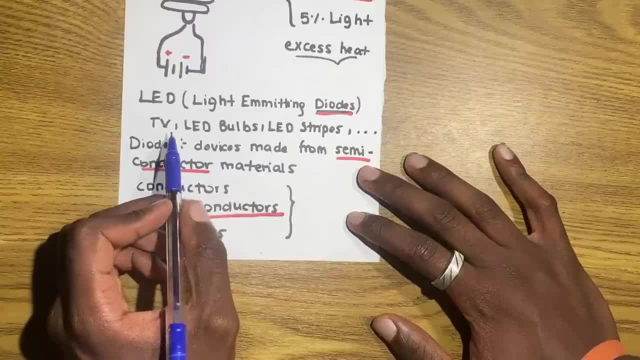 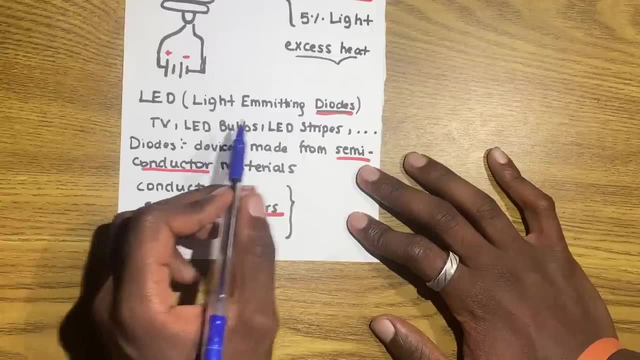 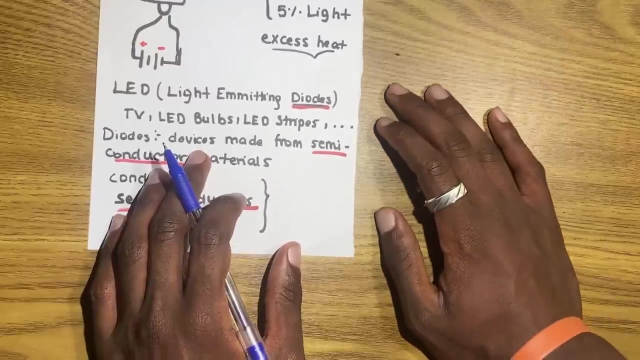 light emitting. it emits light. What is the word diode? Let's check it out right here. So, before checking out diodes, LEDs are something that we use day to day. We have LED TVs, LED bulbs, LED stripes that we put inside of our rooms to just decorate, and all that. So LEDs are something. 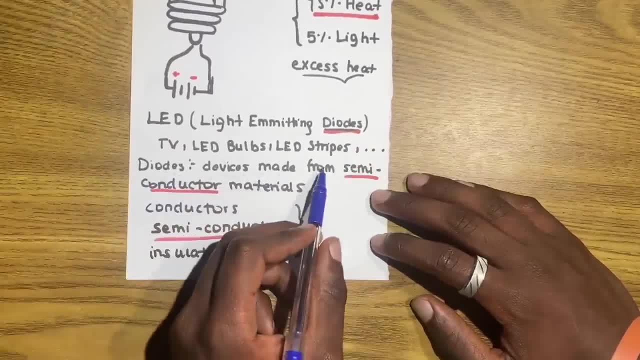 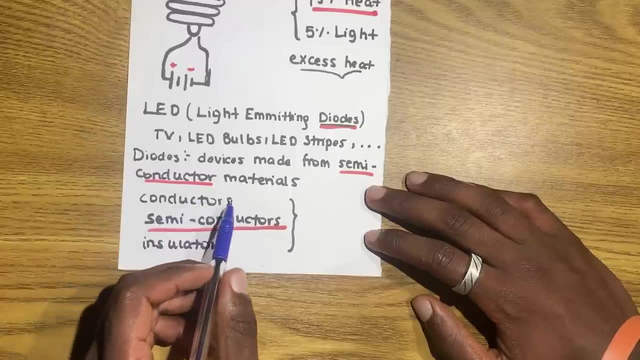 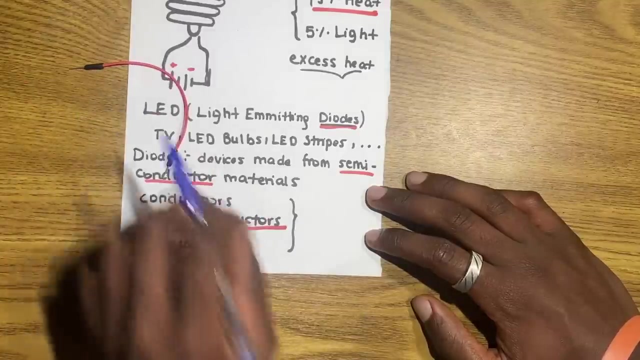 that we use every single day. Okay, So what are diodes? Diodes are devices made from semi conductors. Okay, so we know conductors and we know insulators. Conductors are what? Conductors are materials that can conduct electricity. For example, we can take this wire: It's a conductor. 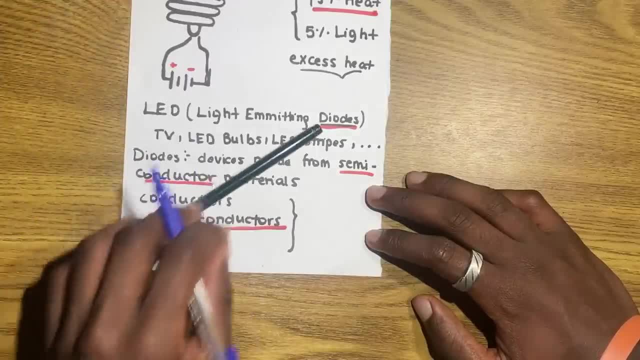 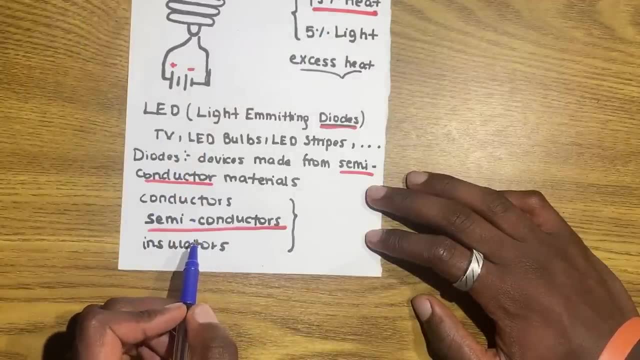 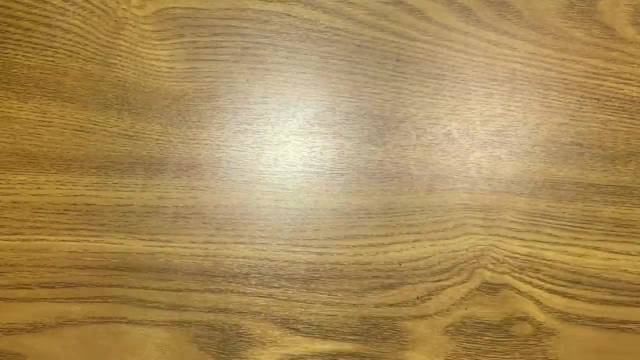 Okay, so we have insulators too. Insulators are the ones that are incapable of conducting. for example, let's take this pencil that is just made of newspaper and in the middle we have semiconductors, so they show the property of conductors and also insulators. so let's check. 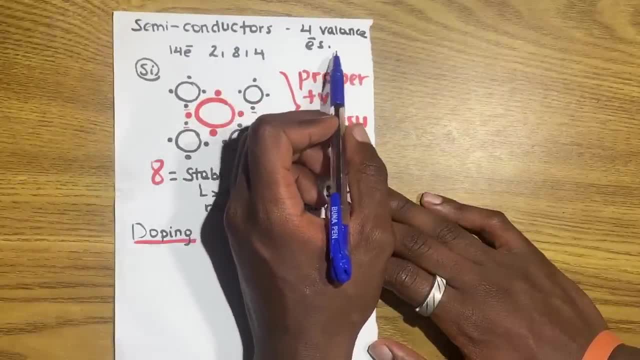 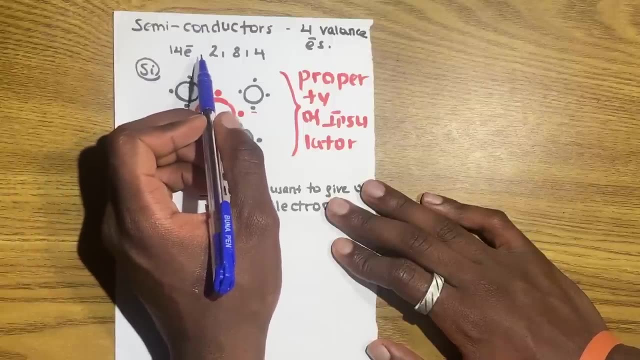 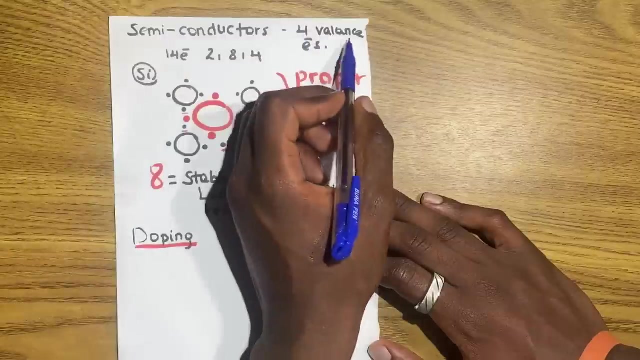 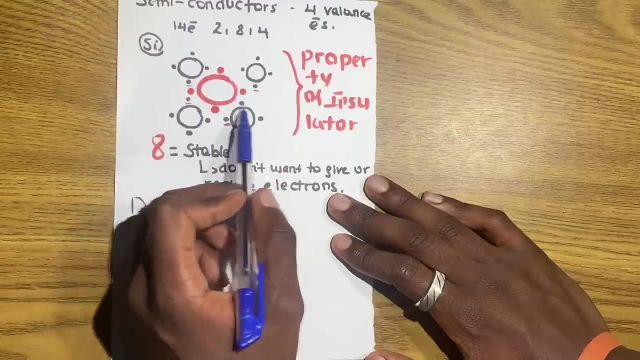 them out. when it comes to semiconductors, they have four valence electrons. so let's take as an example, let's take silicon. it has 14 electrons. when we arrange it it becomes two, eight, four. so it has four electrons on the outer shell. so it's obviously four valence electrons, right here. 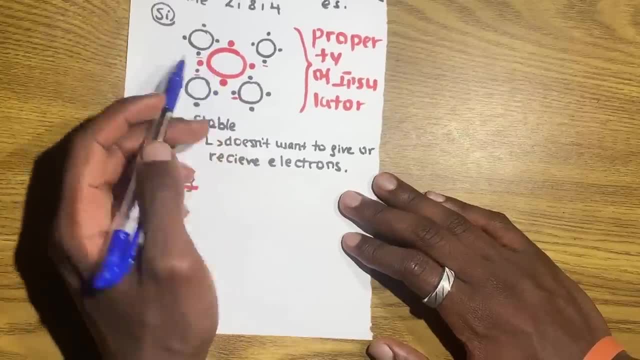 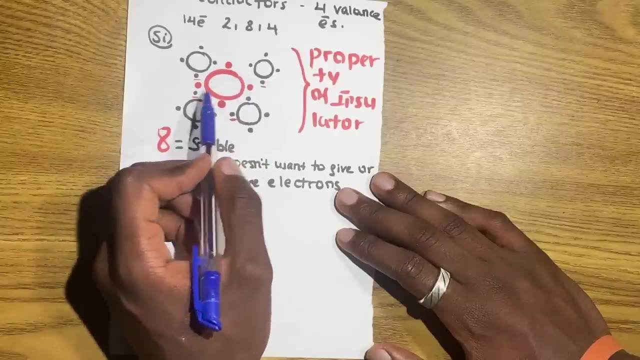 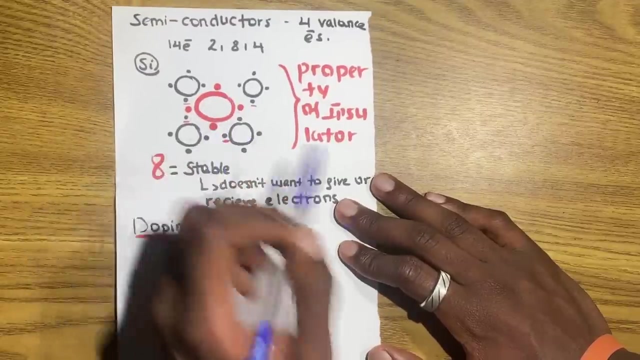 so when we align five silicon atoms, we have five silicon atoms right here. okay, so when we put them in such a way, they become stable. let me explain. so, at the center, the one with the that is marked with the red, the center molecule, and it has four valence electrons. the electrons are represented with dots, as you can see here. 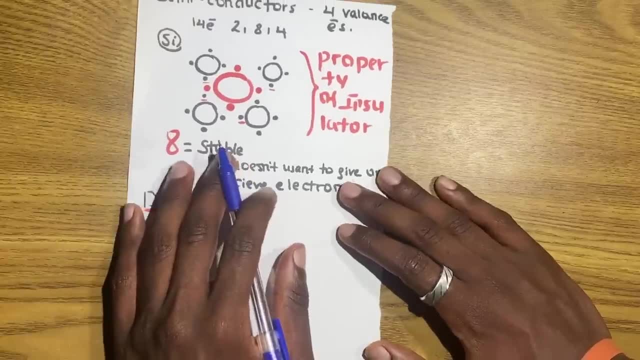 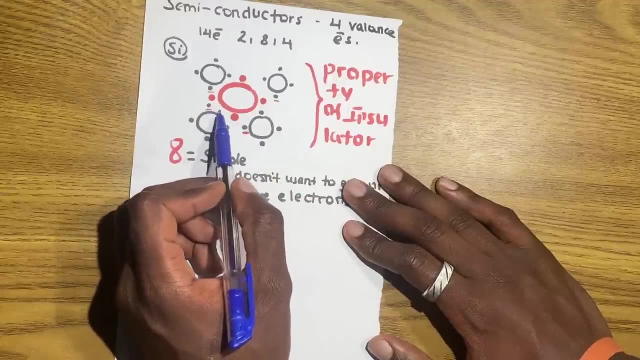 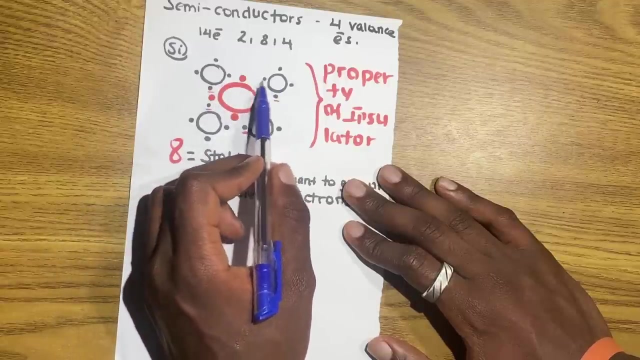 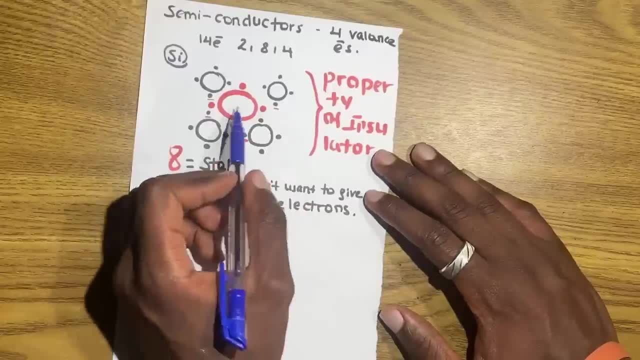 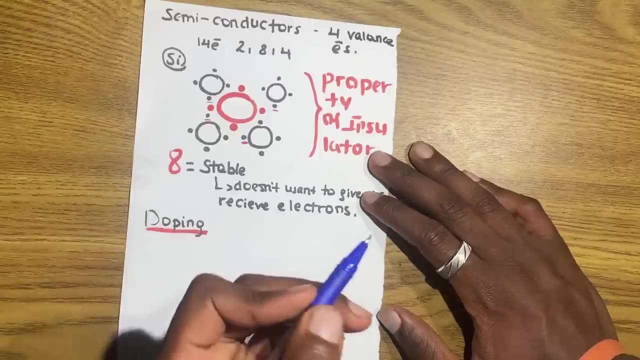 silicon atom and the central atom, this silicon atom and the central atom, this silicon atom and atom and the central atom. so if we add up the electrons right here, we have one, two, right here, three, four, and we also have four that we already have right here, four valence electrons that we 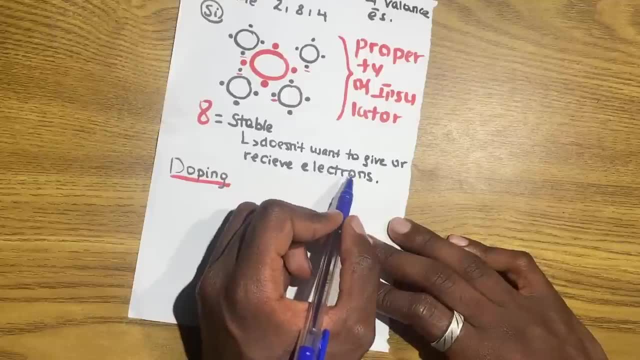 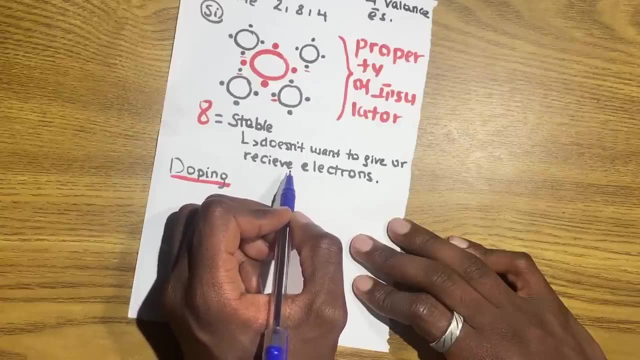 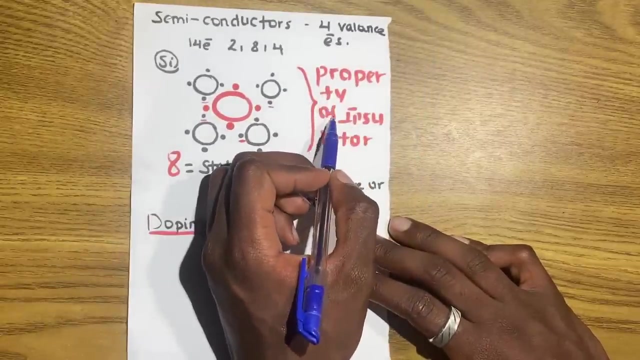 have from the beginning. so when we add four plus four it is eight. so in this case it's stable. so it doesn't want to receive or give any sort of electrons. so in this case it's not going to conduct electricity. why is that? so there will not be free electrons to move, so current cannot flow. 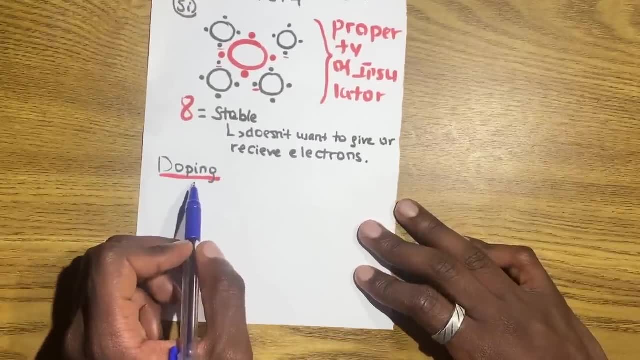 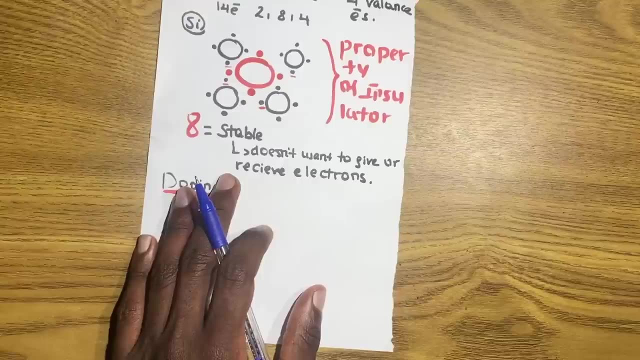 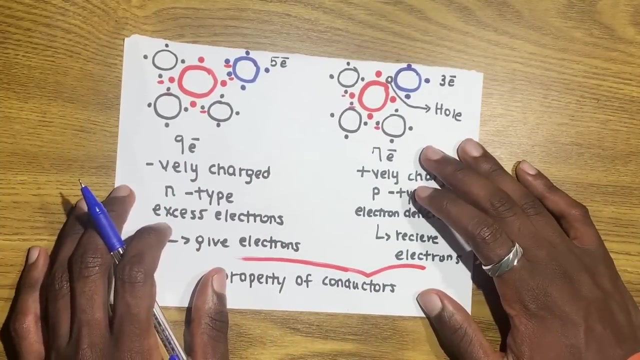 okay, so it shows the property of an insulator right here. so right now we're going to use a method called doping, and this is the method that actually changes semiconductors- and just the gain for semiconductors- and actually makes them behave like conductors. so let me bring this: 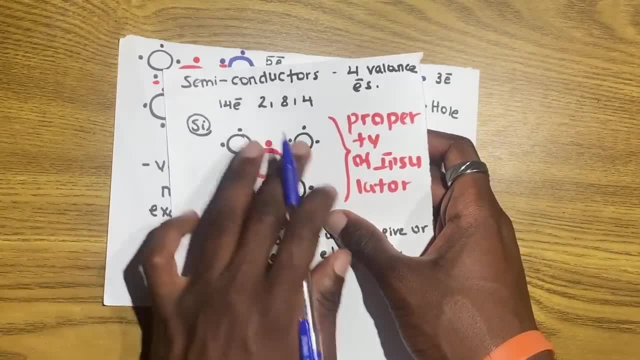 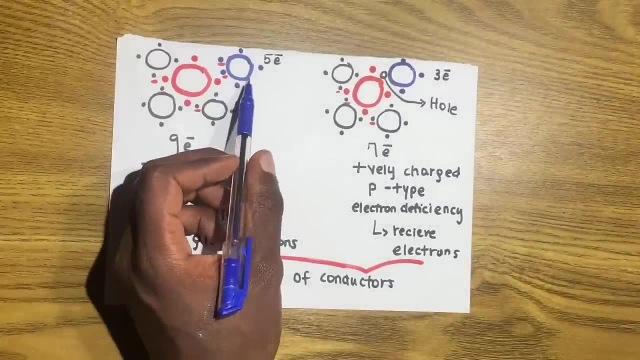 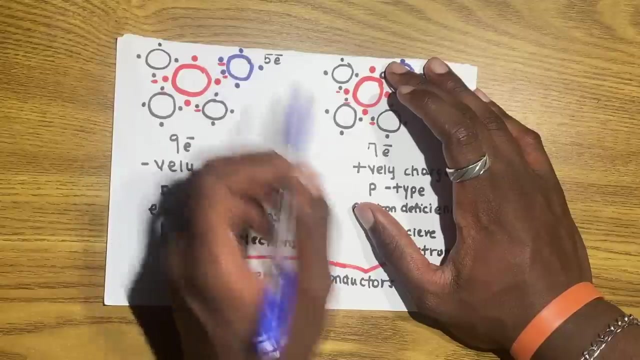 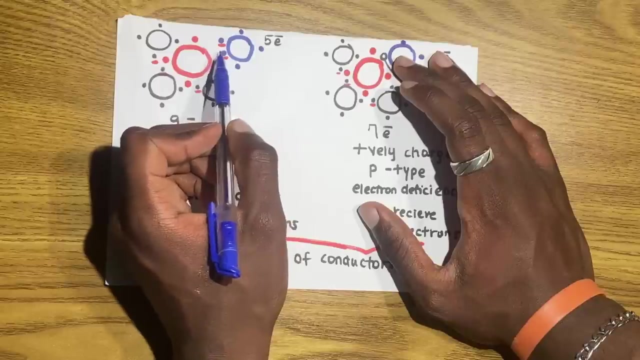 right here. we can check it out right here. so earlier, if you'd actually look at it right here earlier, we had five silicon atoms. okay, instead of having five silicon atoms, replace that one silicon atom right here, we're going to replace it with an atom that has five valence electrons, so it has five dots right here. so instead of giving one like 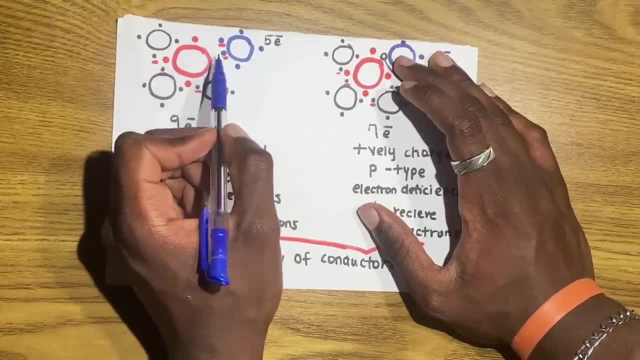 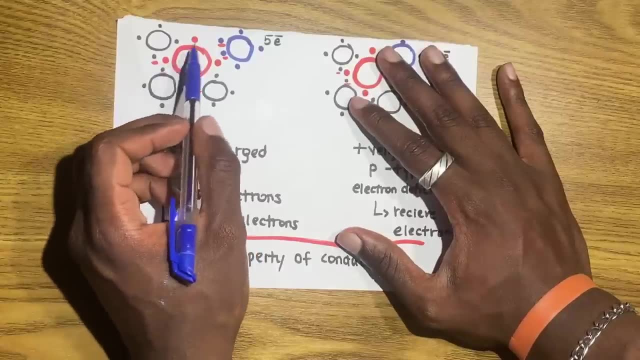 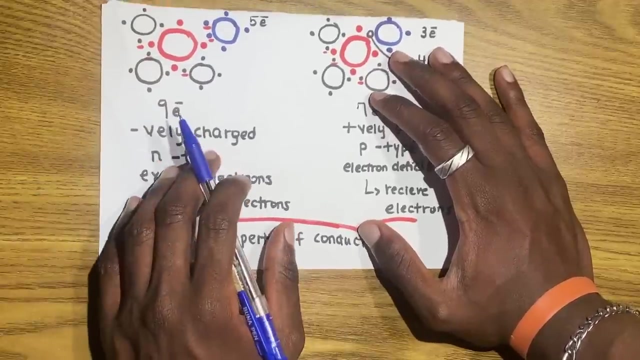 every silicon atom right here, it gives two. so we're going to have instead of eight, we're going to have nine electrons. we could even count it: one, two, three, four, five. we have five shared electrons and we have four valence electrons that we already have on silicon atoms. so when we add that up becomes nine electrons. so in this case it is. 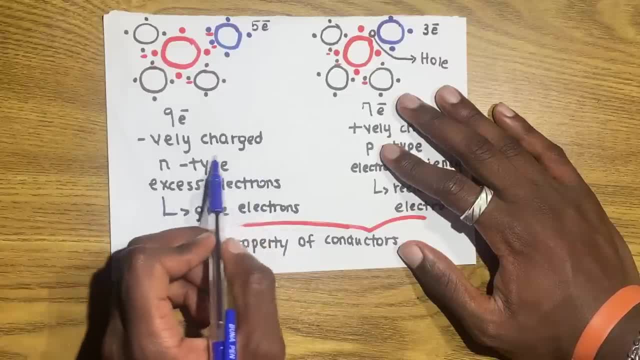 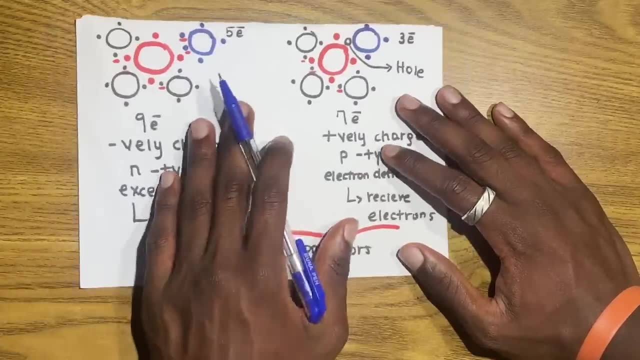 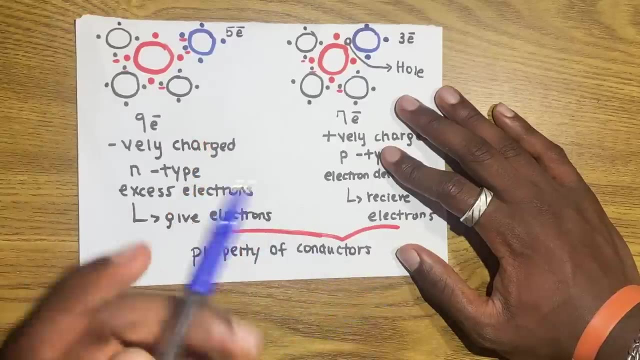 negatively charged because it has excess amount of electrons right here and it wants to give those electrons, so it's negatively charged. that's why it's called the n type, n standing for negative, okay. so right here we're going to conduct electricity, because we have excess amount of electricity. we 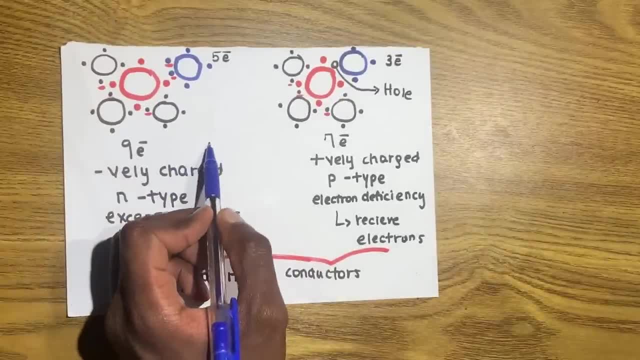 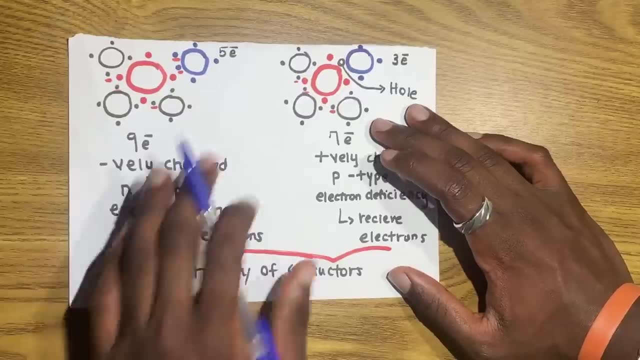 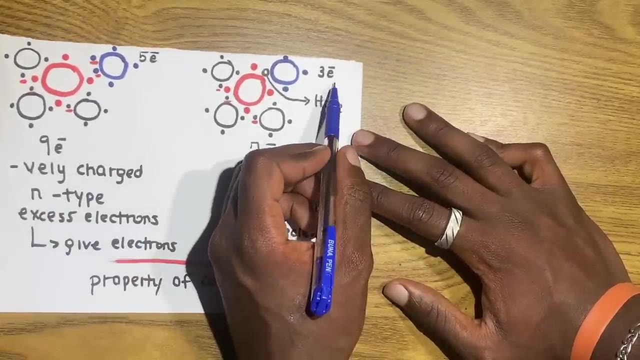 have free electricity. you have that one electron that wants to what, that wants to move freely, and again we want to go back to what? to eight electrons. okay, we want to be stable. so in this case, what do you want to do? we want to give electrons. so right here it shows the property of a conductor. we can. 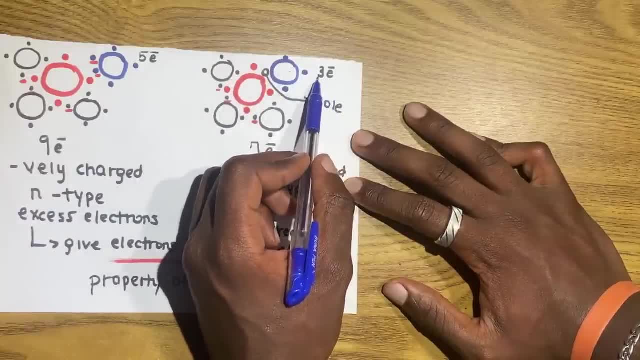 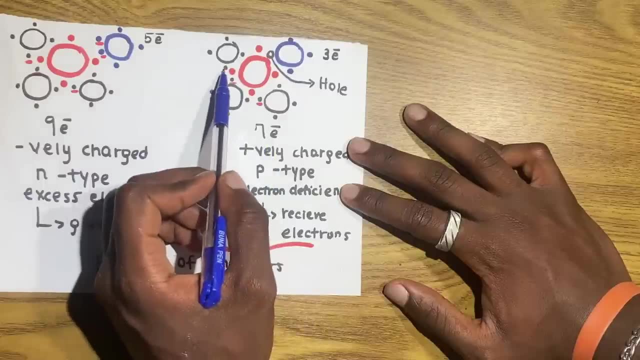 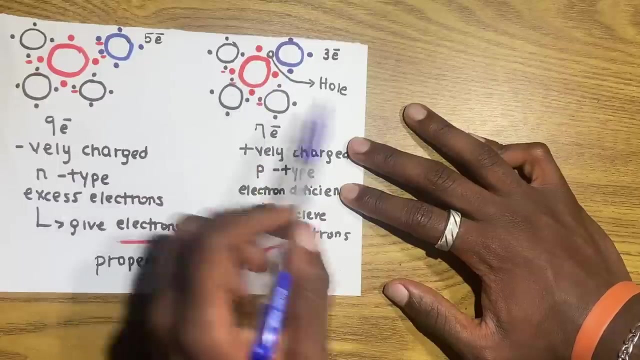 also use another method. in this case we're going to give it three electrons, so we have four silicon here. the one marked with blue is going to be the three electron element. so right here, when we add all this up, we're going to have seven electrons. we have one, two, three electrons that are shared and we 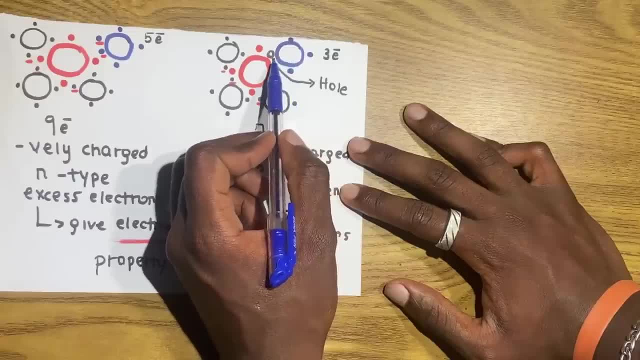 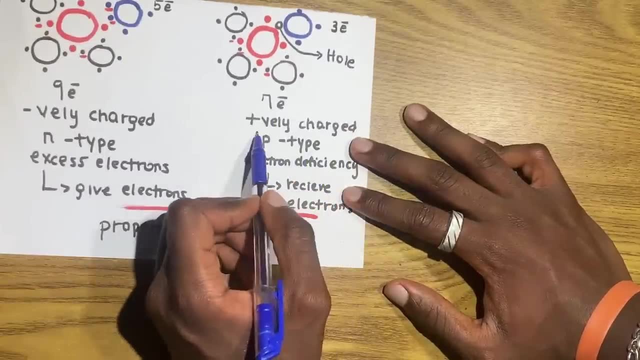 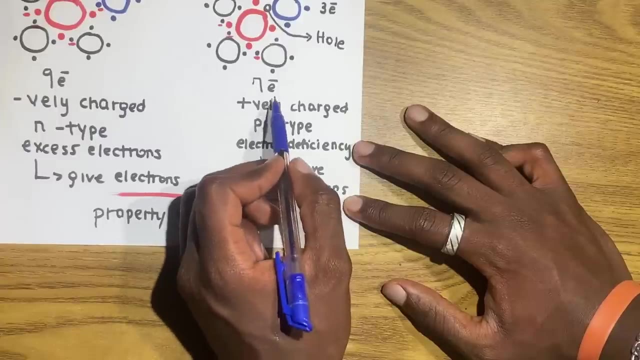 have four electrons that are again a silicon atom. so when we add that up it becomes seven electrons. so this will not contribute towards any shared electrons. this element right here that has three electrons. okay, so in this case we are positively charged. okay, is that? so we have an electron deficiency and we want to what receive electrons because we 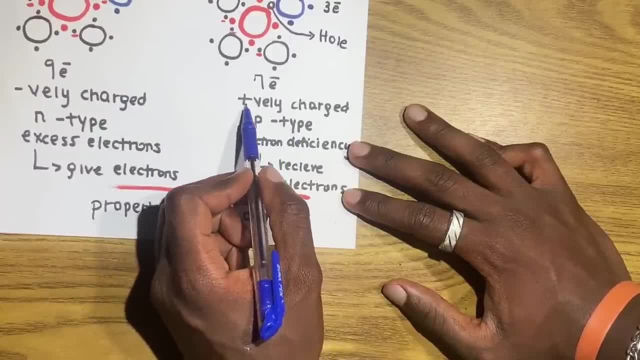 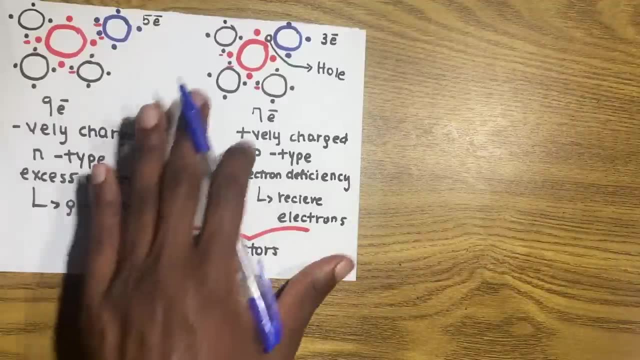 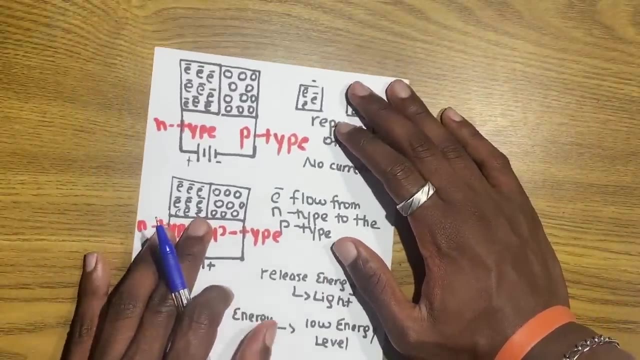 want to achieve stability with eight electrons. okay, so it's called p-type p, obviously standing for positive. okay, so this is what is going to basically happen, and one thing that we're gonna finally need to check is this: okay, so, with that in mind, right here we have. 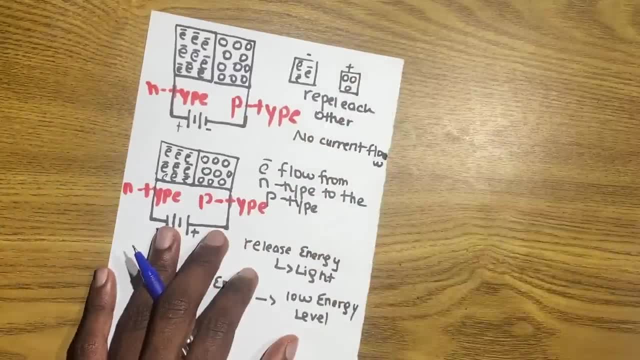 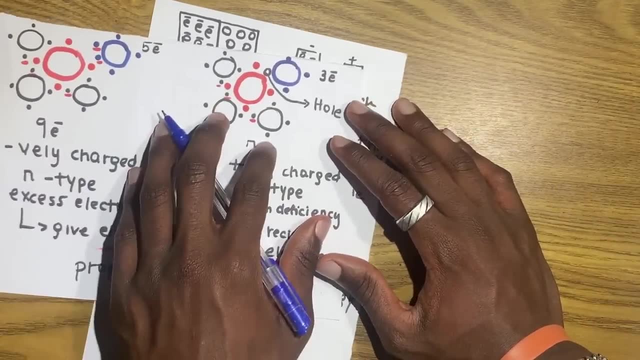 p-types right here that have excess amount of electrons, electrons, electrons and electrons right here, and we have the p-type that have holes. so let me discuss the concept of holes and what they are. if you look right here, we have hole. a hole is basically an empty space. 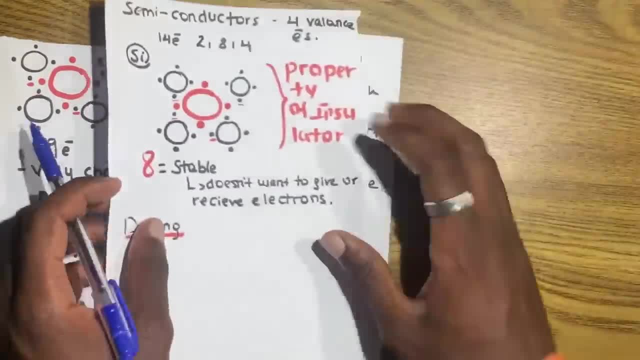 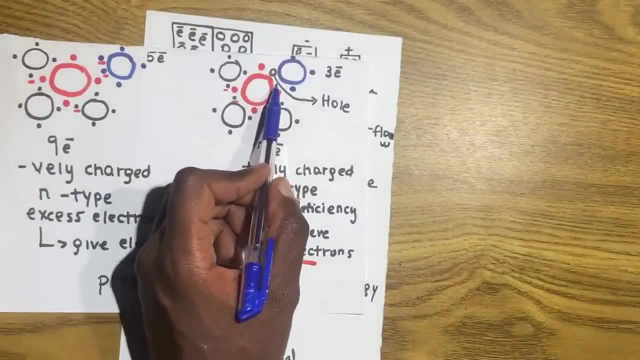 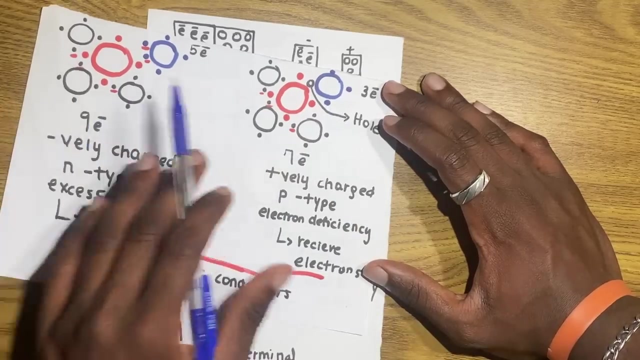 an empty space where an electron should have been. so if there was, let's say, four electrons, like earlier, like we had right here, like pad right here, exactly right here, we just put the electron. but right now what we have is an empty space because we don't have an electron. so 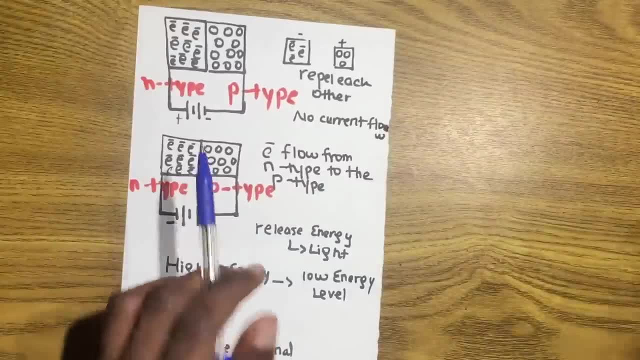 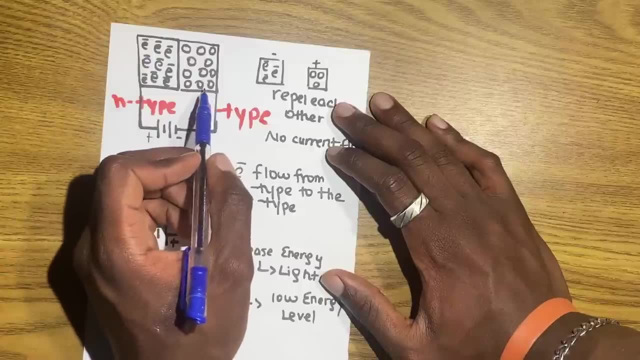 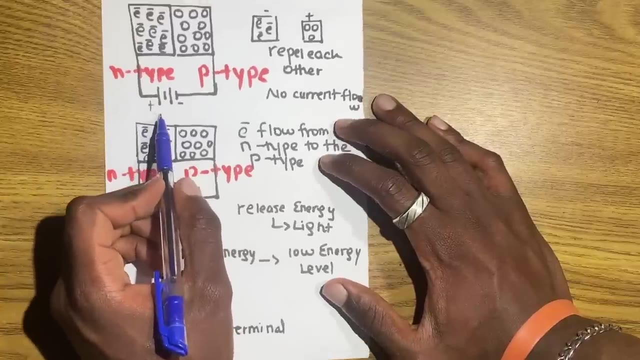 basically, holes are just representation of just empty spaces where an electron should have been. okay. so right here, in the n-type, we have electrons over electrons over electrons, while in the p-type, in the p-type, we have holes and holes and holes and holes. okay. so right here we connect the. 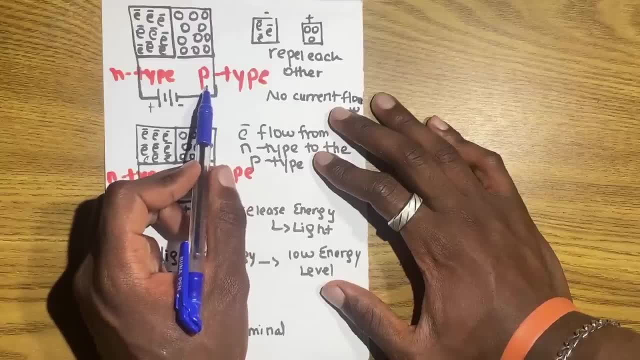 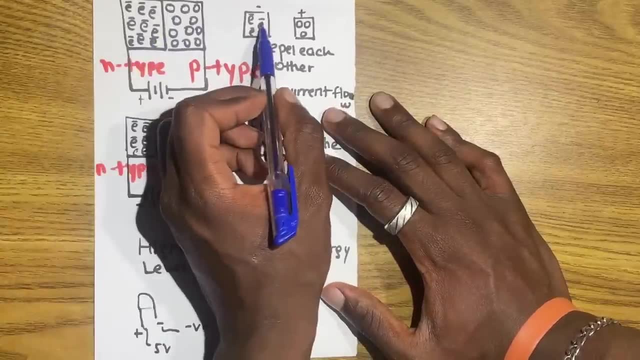 positive terminal of the battery. as you can see right here, with the n-type we connect the negative end of the battery with the p-type. in this case, what basically happens is from the electron actually going towards the holes. what's going to basically happen is they're going. 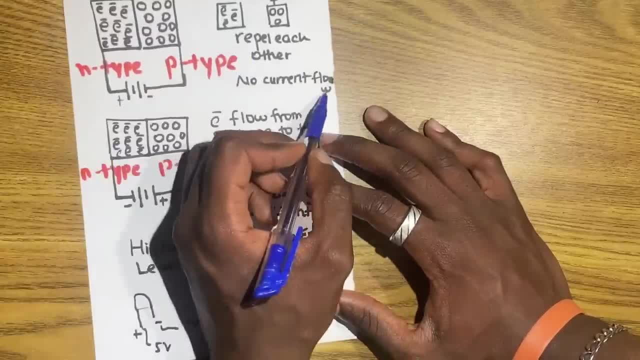 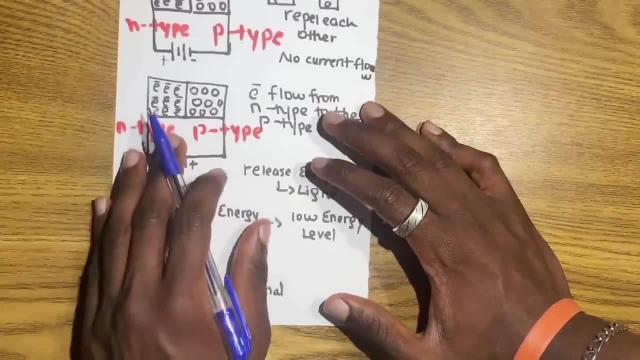 to start repelling each other. so this one is negatively charged and this one is positively charged, but they start to repel each other. so in this case, current will not flow. okay, so we connected the positive with the n-type and the negative with the p-type. but right now, when we 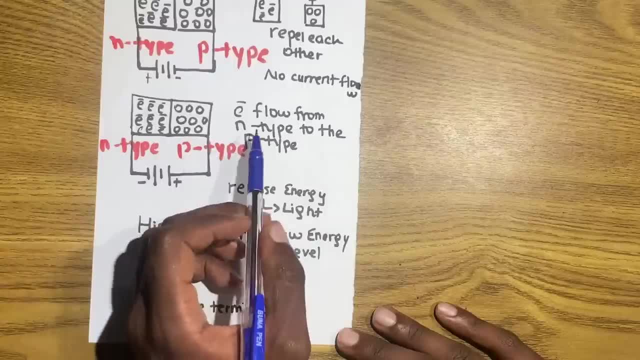 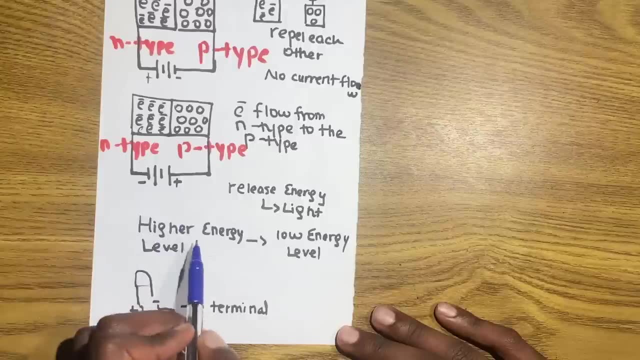 change the direction of the battery and we connect the negative with the n-type and the positive with the p-type. what basically happens is electron flows from the n-type- the p-type, so this electrons flow from n-type- the p-type, so in this case they're flowing. 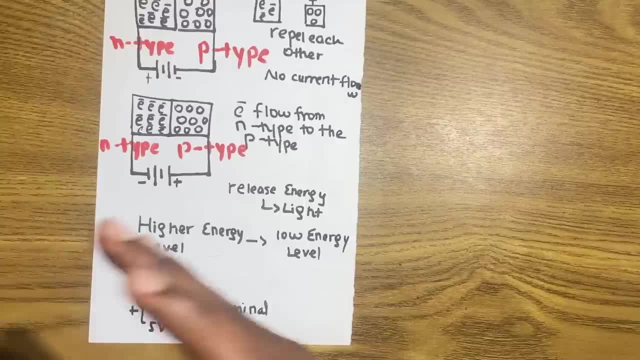 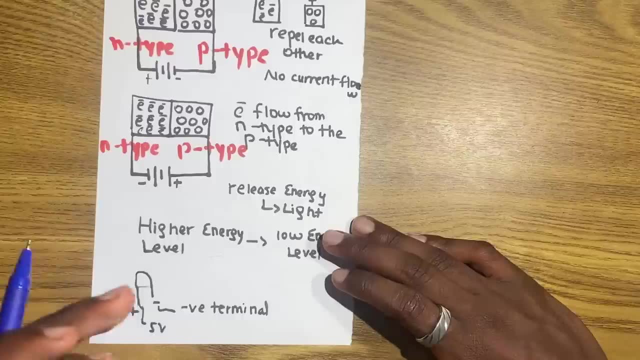 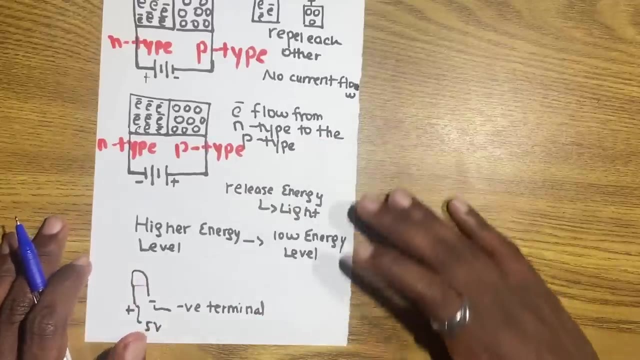 from higher energy level to a lower energy level. okay, so in this case, when they're flowing, when electrons are flowing from higher energy level to a lower energy level, they're basically going to be releasing energy and, as you know, the rule of conservation of energy. energy is neither created or destroyed, but rather taken from one form to another. so when they release, 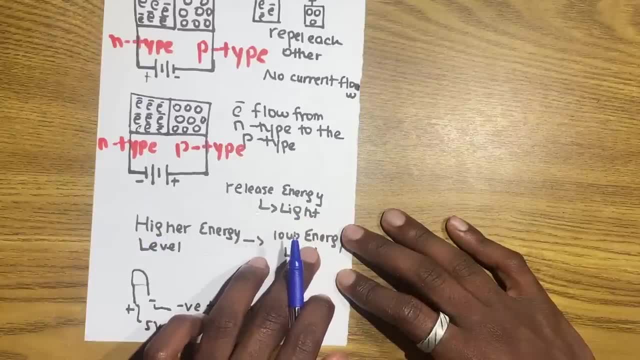 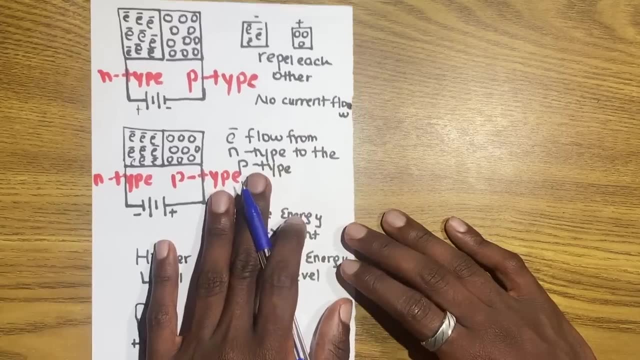 that energy, the electrons. they release that energy in the form of flight. so when they move from higher energy level to the lower energy level, they'll be losing energy, and that energy that they're going to be releasing is going to be in the form of flight. so right now, what basically happens is: 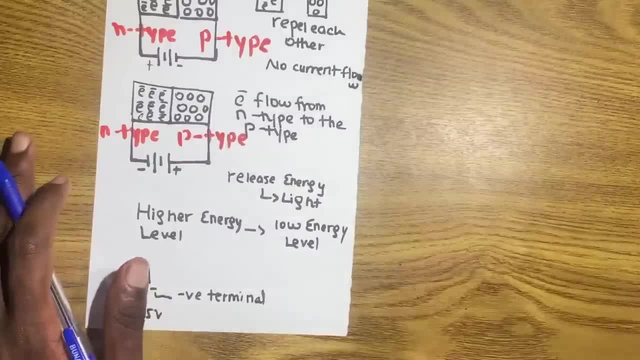 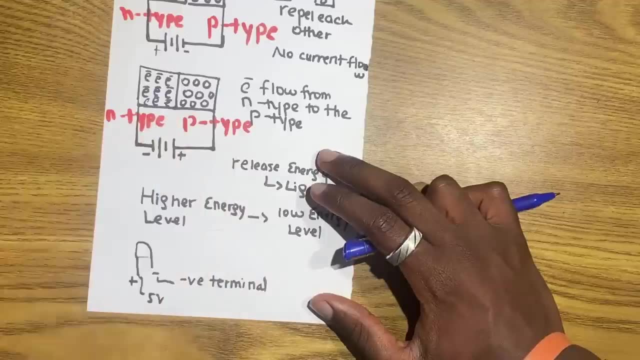 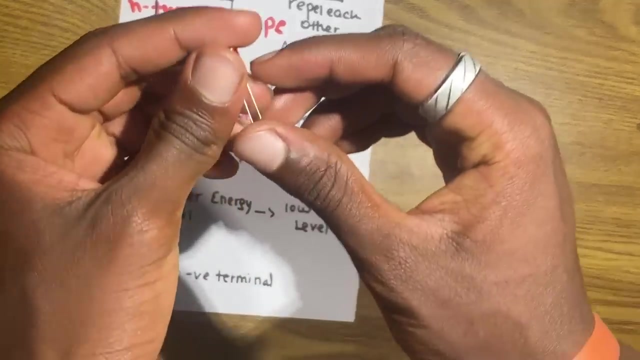 we directly change electrical energy directly to light energy, so we don't need to have, you know, excess heat and all that, like light bulbs did. okay, so you might be wondering then, what is the p-type of, uh, you know, an LED? look like that in real life, because it matters like what part of 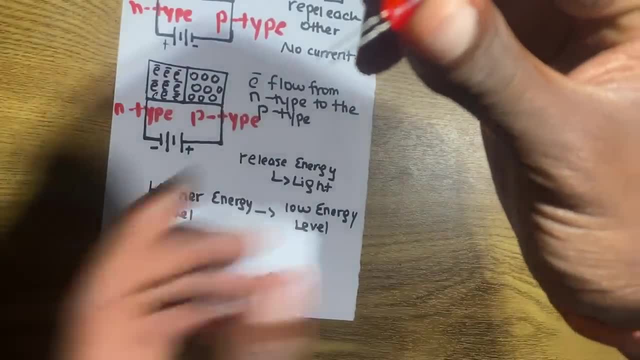 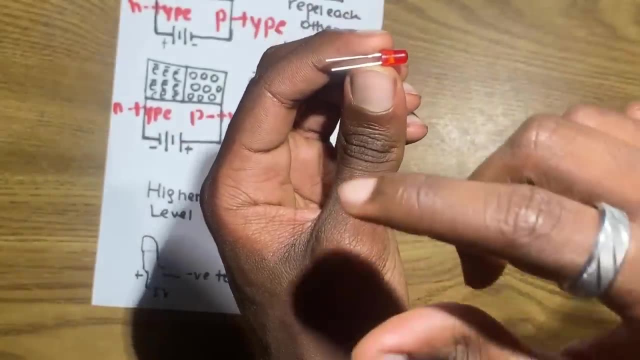 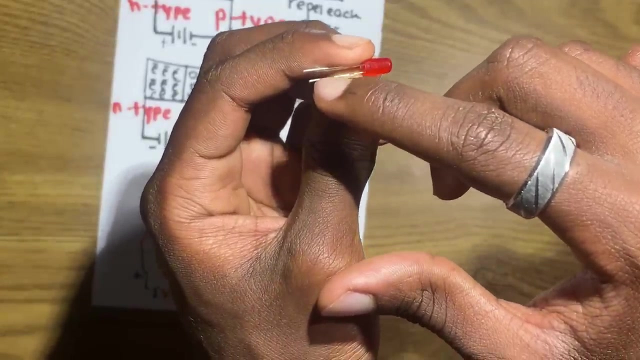 the battery that you connect it to. so if you look at your LED right now, let me just bring it up close to look at it right now, let me just actually let me get this okay. so if you look right now at your LEDs, the LED legs right here, they're not even. one is longer and one is shorter, okay. 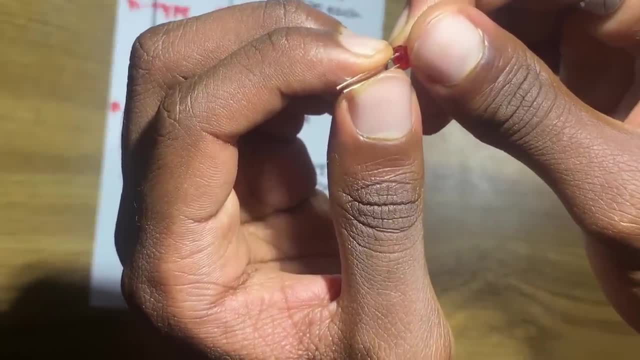 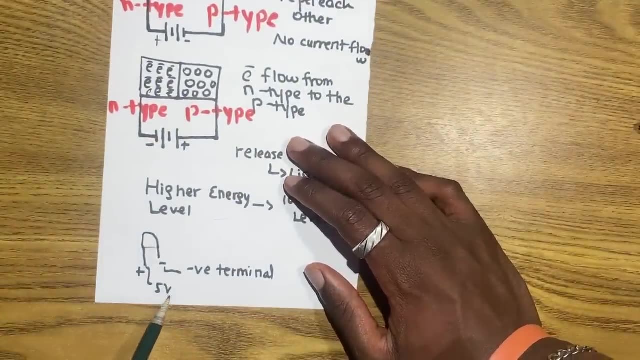 so the longer one, the longer one. if you look right here, the longer one is the positive and the shorter one is the negative. the longer one is the p-type, while the shorter one is the n-type. okay, so if you look right here, we're going to connect the positive end of the battery right? 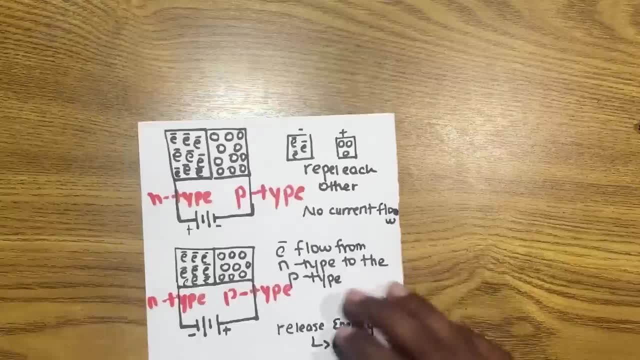 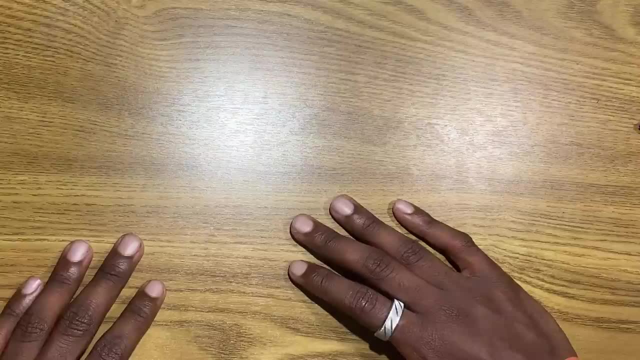 here with the positive, the longer side right here and the negative part of the battery with the negative terminal. okay, so we're going to actually check, uh, the next section on how to actually assemble our components that we've learned so far. so see you in the next section. 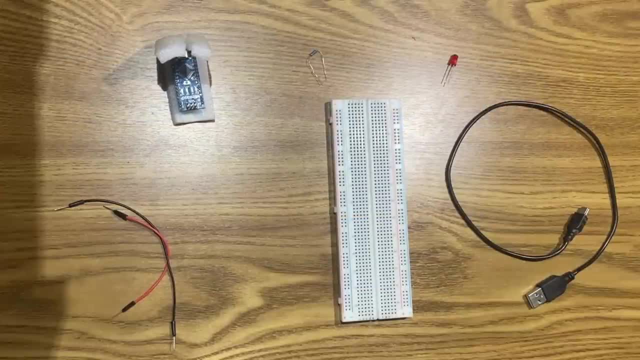 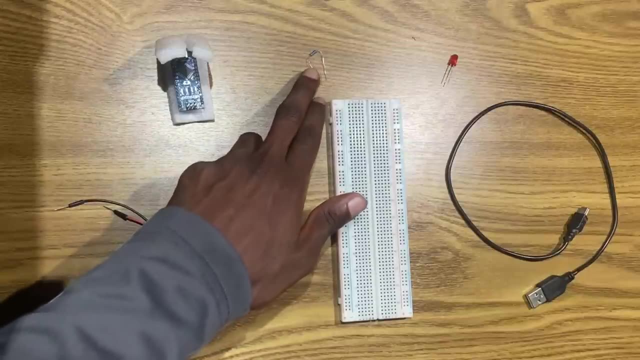 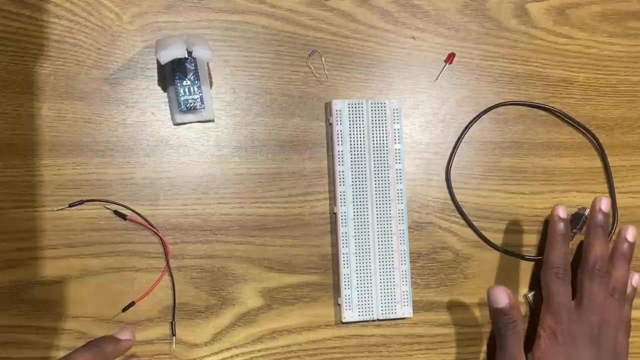 so now we're actually going to be in the exciting section of actually building and assembling what we've learned so far. so we have our Arduino right here. we have our resistor, which is again recommended to be 300 to 400 uh. we have our LED right here. we have a connecting USB right here I'm going to be connecting, uh, my 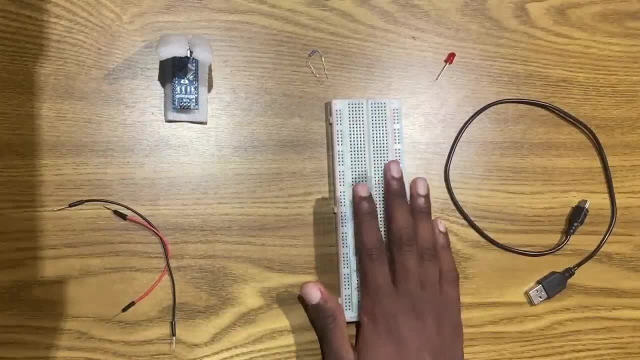 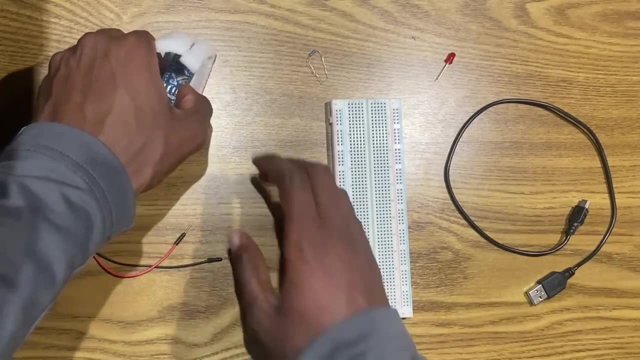 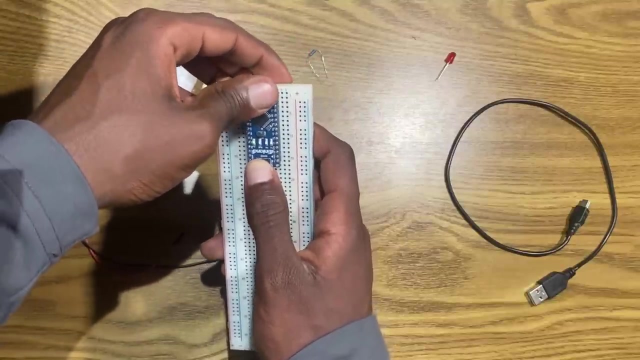 Arduino to a laptop and I have my Arduino breadboard right here, okay. and then I have my connecting wires- okay. so let me begin by connecting the Arduino with the breadboard. if you have an Arduino Uno, you don't need to connect your Arduino with the breadboard. 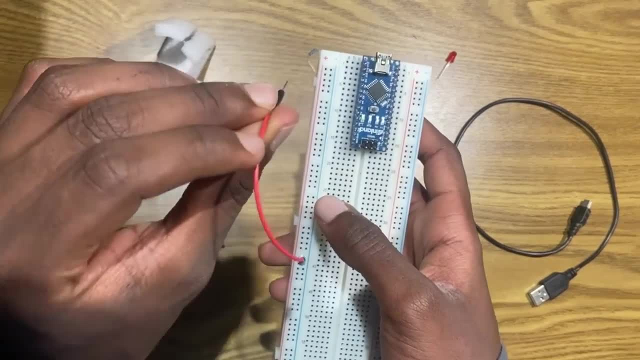 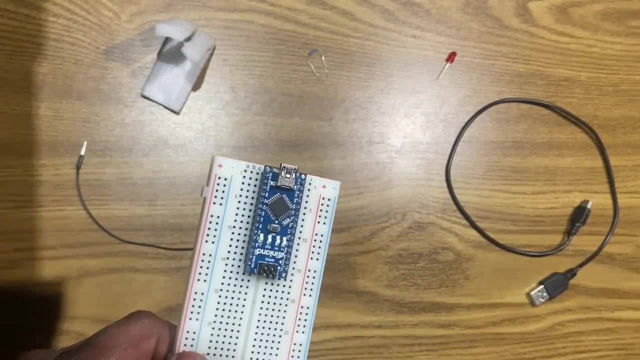 all you need to do is a hole again, so all you do is again connect it directly to a connecting wire. okay, so second thing I'm going to need to do: we're trying to build a circuit actually, so let me bring the circuit right here. okay, so we've got our Arduino connected. you want to connect it to the? 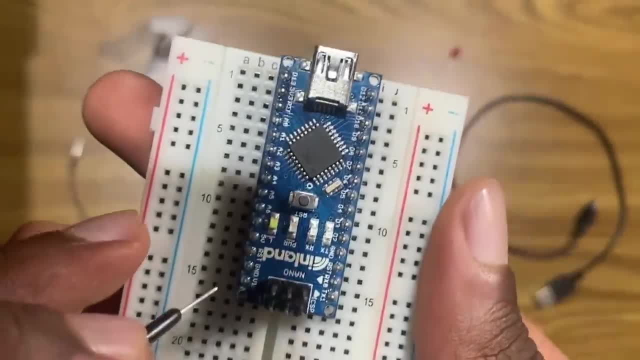 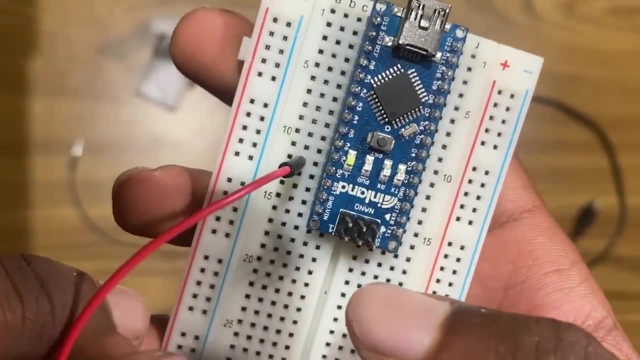 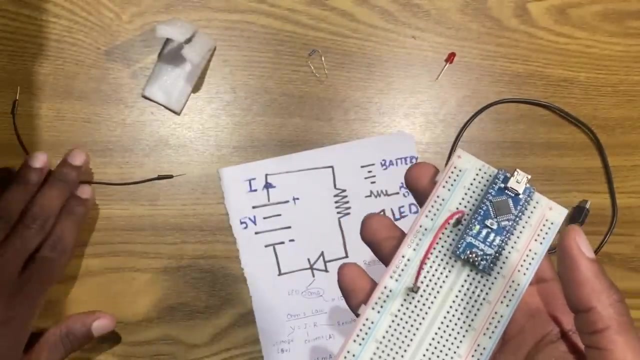 5 volt. so let me go right here and let's try to connect the 5 volt. there's the 5v, connect it right there to the 5 volt. okay, let's say, put it around 25.. okay, let's put it randomly on 25.. then now what we want to happen. 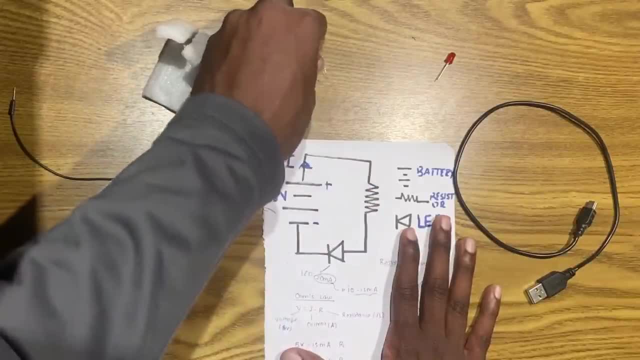 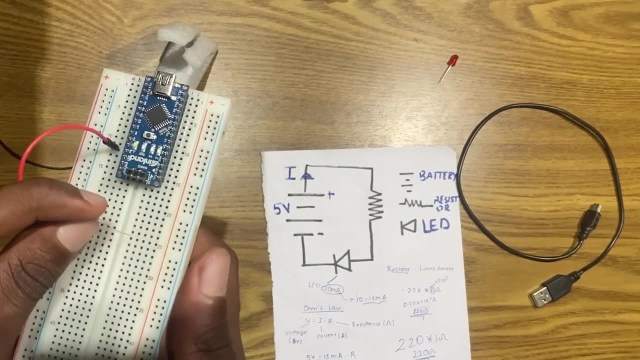 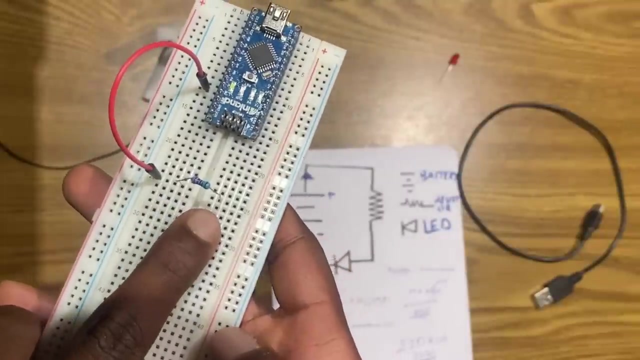 is we want to connect it to a resistor. okay, so let me bring my resistor right here, bring it right here and let's let me just try to connect it a bit, if you can see it, okay. so one thing you notice is I connected it across. so, as you remember, 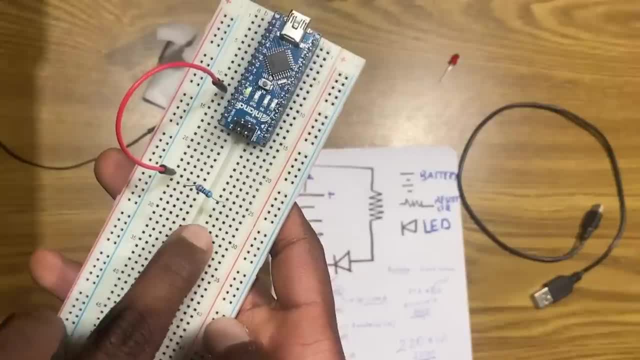 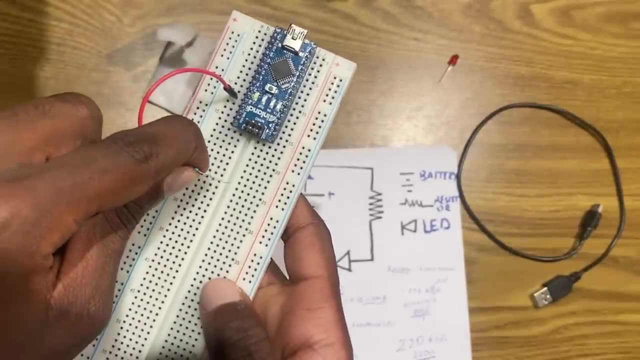 this row is connected. this row is connected, but these two rows are not connected to each other because they have a gap, as I told you guys earlier. so if I connected it, let's say in the same row. okay, horizontally in the same row. let me just make this a bit more thin. 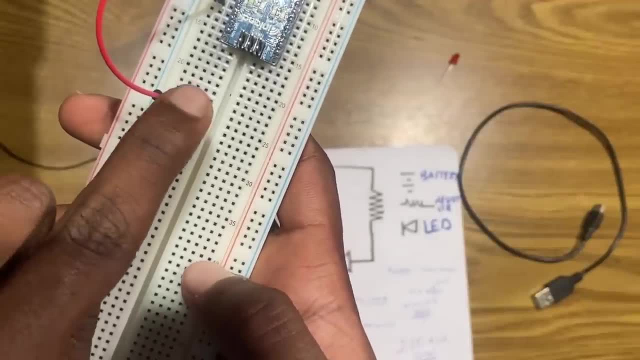 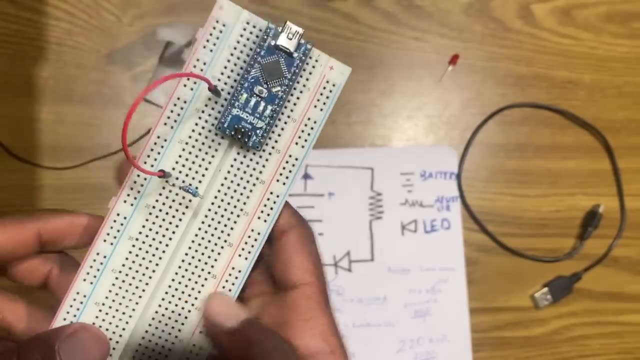 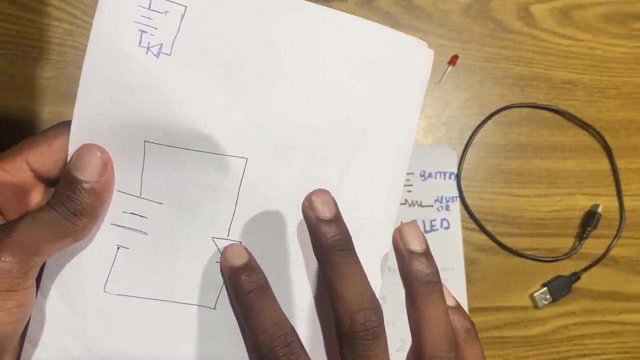 let's say, connect it this way, okay, if let's see the resistor is not connected properly- sometimes this happens- you have to push it in. okay, and if the resistor is not connected properly, what is it doing is basically this type of circuit. we have our again Arduino right here and directly connected. 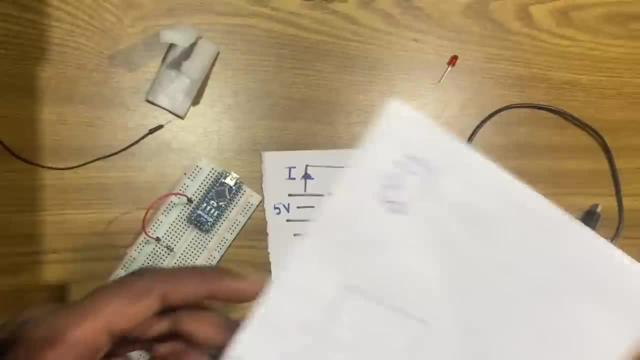 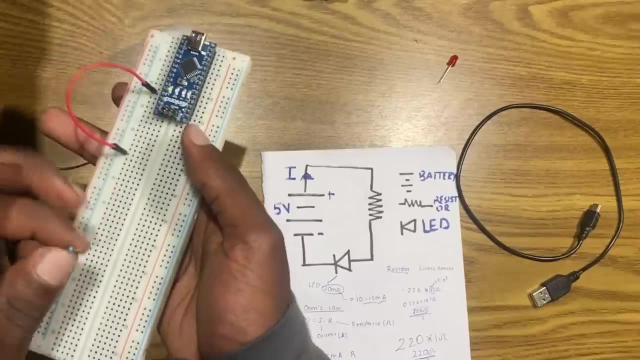 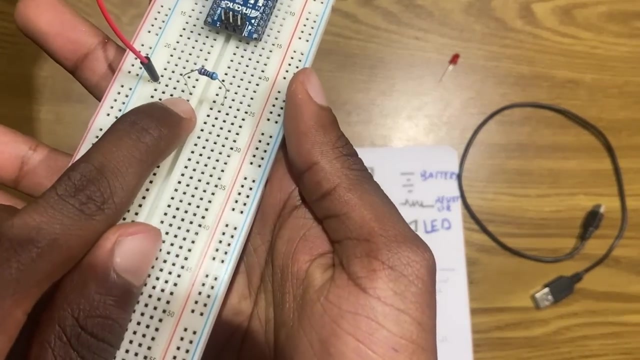 to what? to our LED. so it's going to fry our LED with a one. that's happened again. so if I connected abroad, though if I connected somewhere where it's not connected again, let me just go just make this a bit more wide. it's a bit of a hustle to even connect resistors, to be honest. so you guys can. 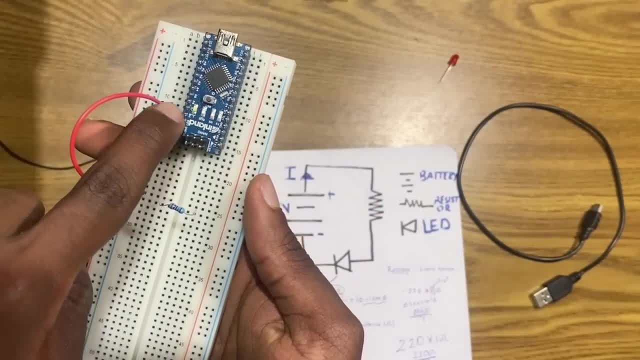 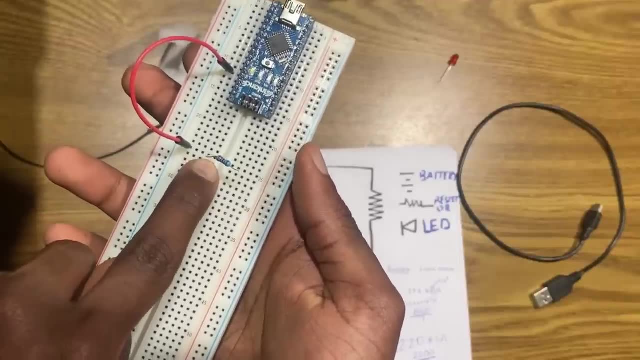 see, I connected it. uh, abroad is current will flow like this: from the 5 volt to the connecting wire goes horizontally and let's see it's not connected right here. what's what is going to basically happen? is it's not going to what conduct electricity? so, at best, at the worst case scenario, if you can either. 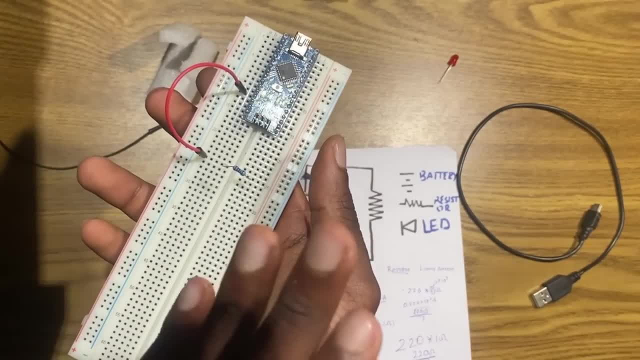 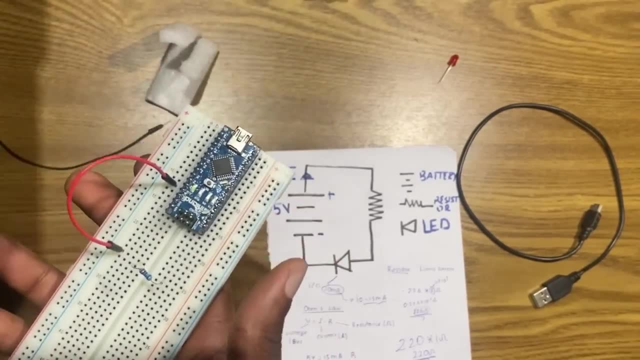 like this is: nothing happens. so the LED does not light up. it's not going to get fried, but it's not going to light up. all you need to do again is connect it properly and um, you're good to go. so we want to connect it. what when you're connecting your resistors? we want to connect it across. if 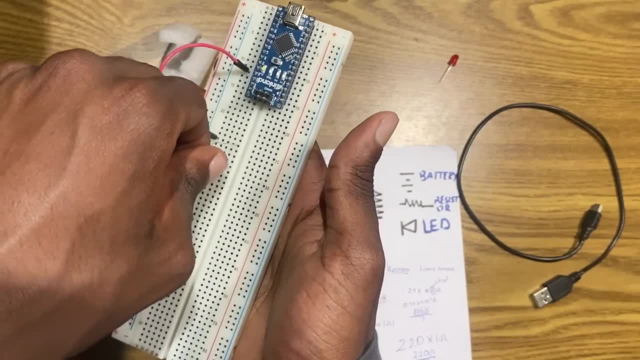 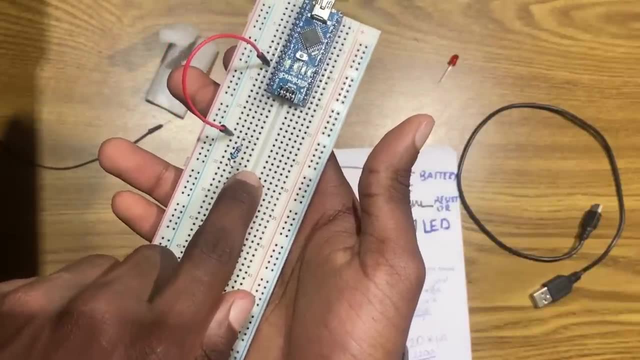 not. we can even connect it vertically, okay, because, again, as I said, they're not connected. so we want this one, one leg to be on the connected side and one leg to be on the side that's not connected anyway with the- again the circuit. okay, with that in mind, 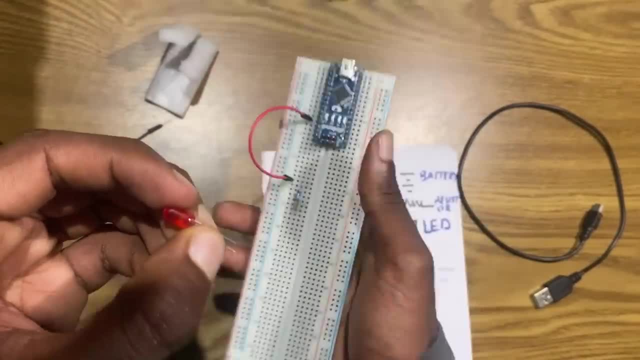 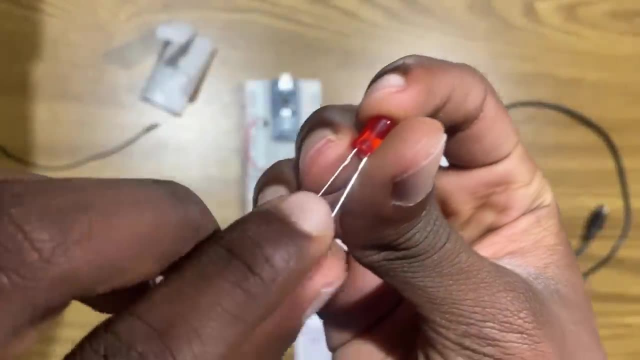 let me just bring my LED and before actually doing that, we first need to identify- let me just make this a bit more wide. we need to identify which one is the positive sign and the negative side. as I've told you guys earlier, the longer side is the positive and we want to. 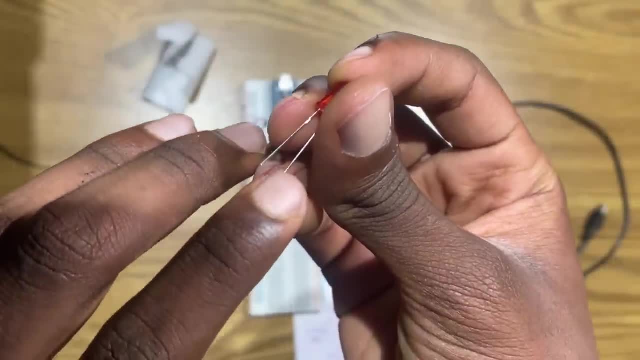 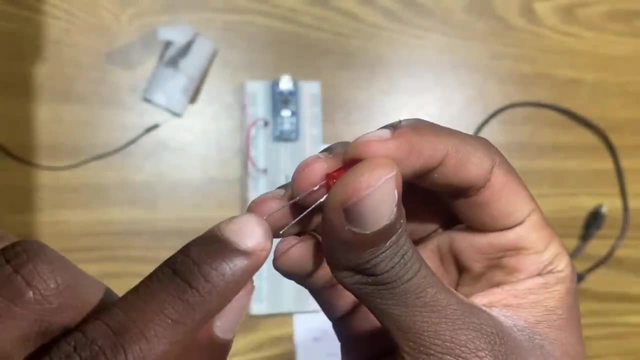 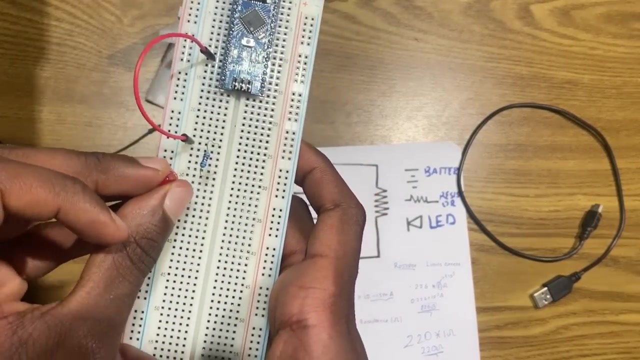 connect it to the positive terminal. as I said again, the P, the P type. okay, this is the P type and we want to connect the negative side with the negative terminal, the n-type. so you want the longer side to be the direction of the positive. so I have the longer side right here and I want 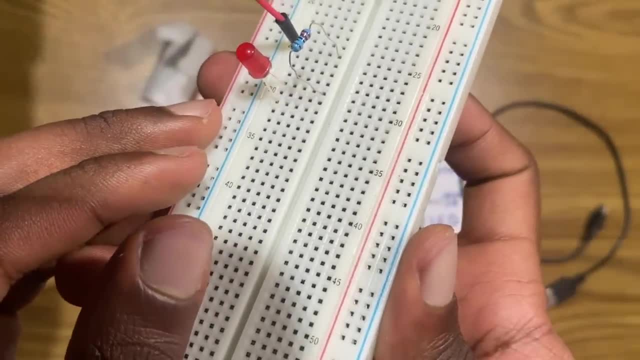 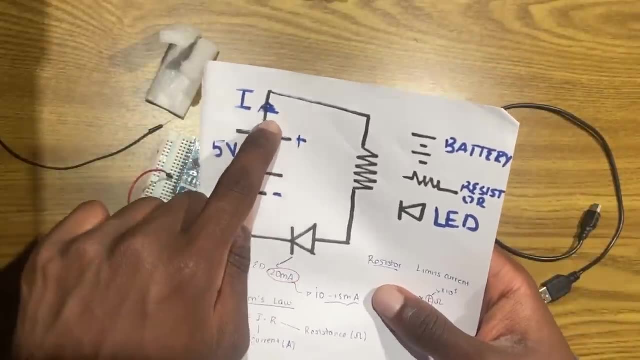 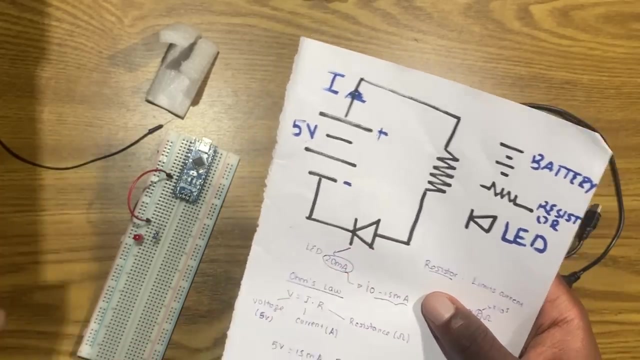 to connect it right here, as you guys can see. okay, now, finally, we connected our Arduino current is, we've connected our resistors. we've also connected our LEDs- the positive side and the negative again. so if you look right here, actually this is the positive side. okay, if you look at it in the 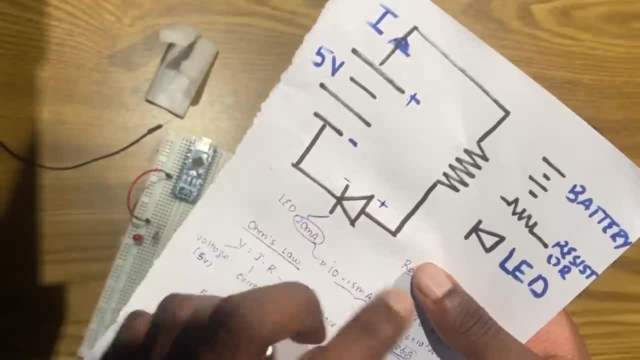 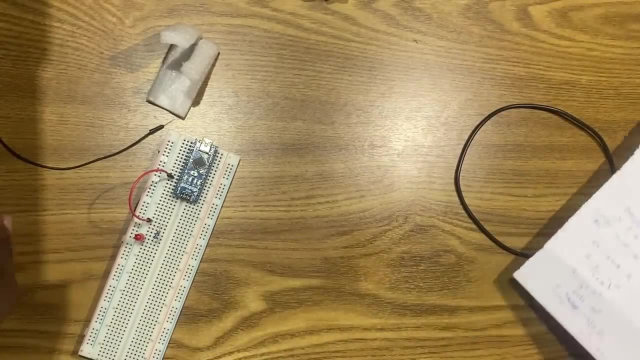 diagrammatically is it's positive right here and we have the negative right here, okay, so again, it's going to go all the way right here and to the negative terminal. and how do we get the negative terminal in an Arduino is? let me go all the way you guys can see it. there's a sign that says g and 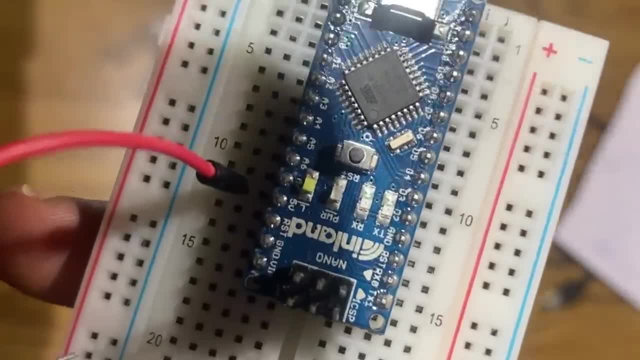 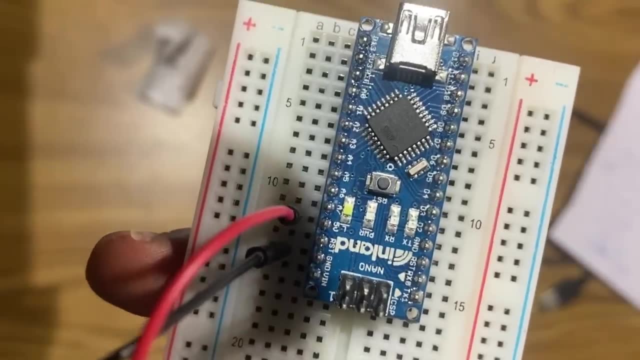 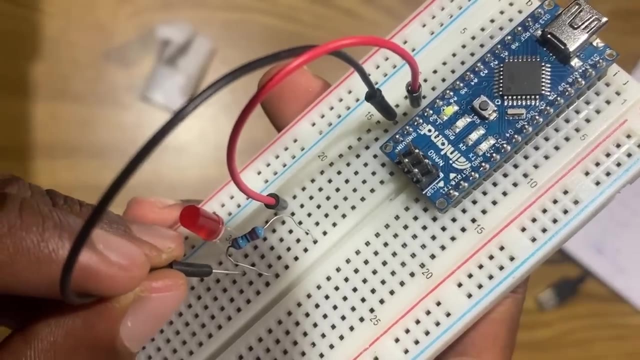 you can see it right here. g and d stands for negative or ground. okay, so if I put g and d right here, that basically means is negative. there's no other meaning towards it. all right, so I want to connect to the negative side of my LED. so all I need to do is push this and we're done building. 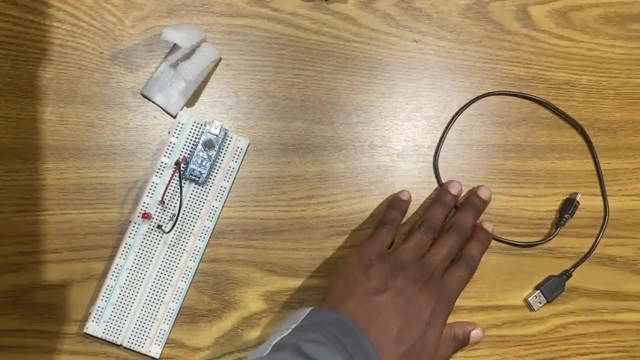 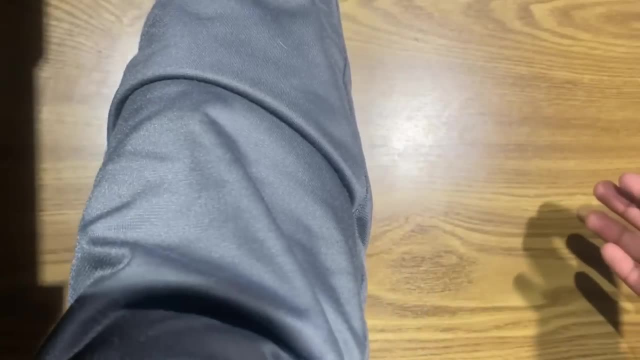 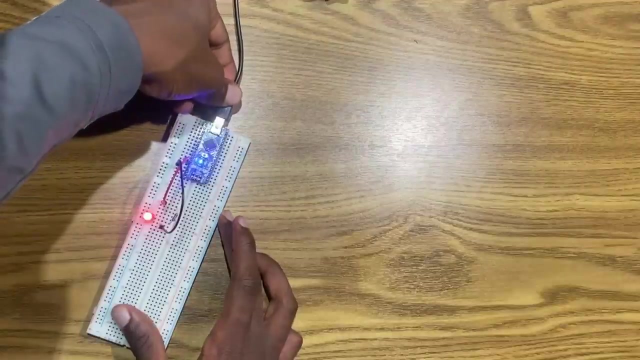 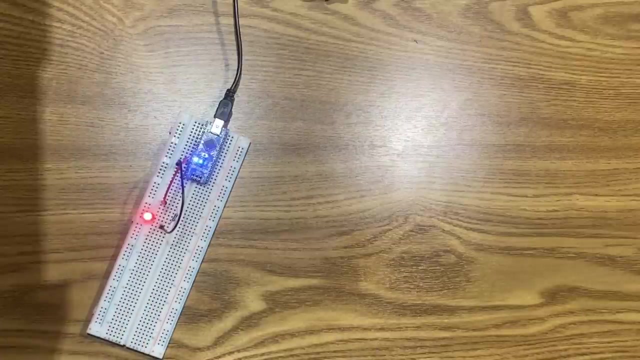 our first circuit. so right now, let me bring, finally, let me finally bring our uh connecting USB, so let me connect it to my laptop. okay, then let me connect my Arduino. there you have it. we have our first up and running LED circuit. let me turn off the light. 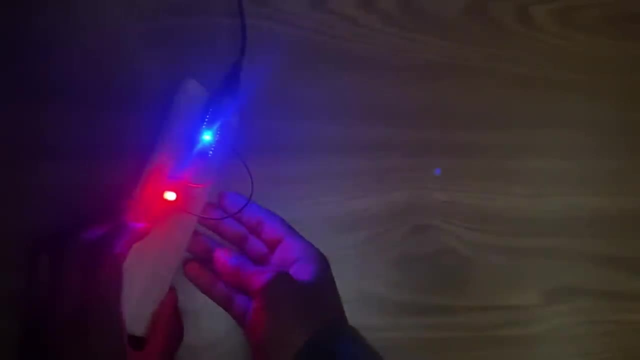 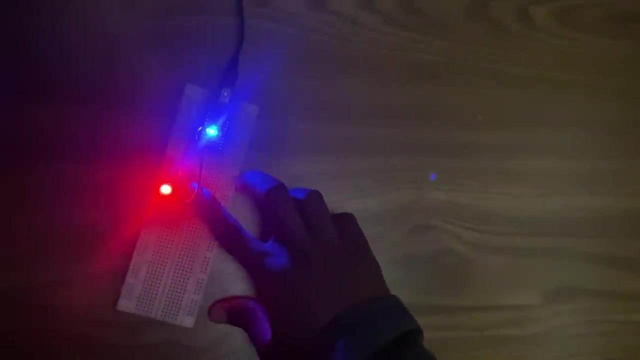 so you guys can see it better. so there you have it again. this is a simple circuit. what's going on? oh, you see the resistors that I was talking about earlier. sometimes they disconnect when we move them again, and what happened was again it turned off, but our LEDs again were not fried, as I said again. 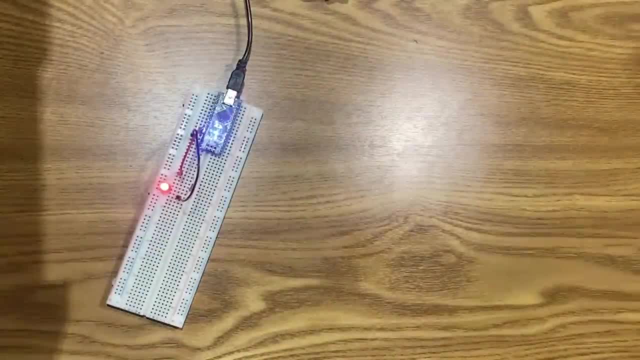 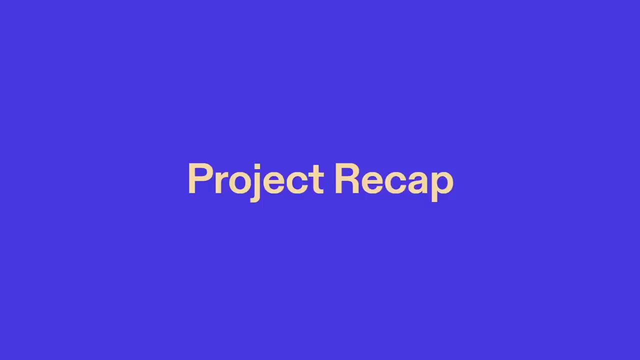 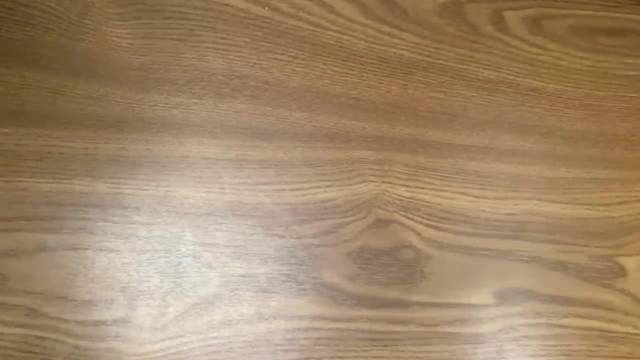 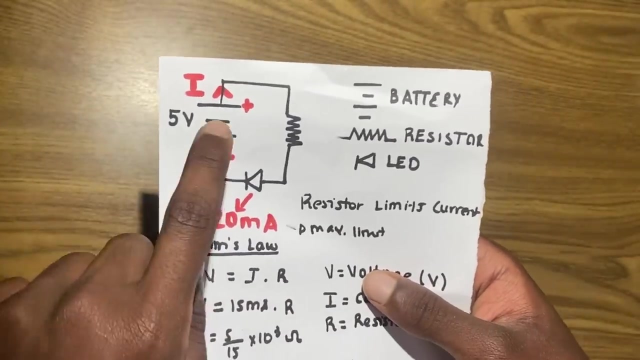 because the current cannot flow through. okay, so with that in mind, uh, see you on the next project. in our previous section, we built a simple circuit that lights up an LED, so let me bring the light right here. so, if we look close enough, we used our Arduino as a power source. 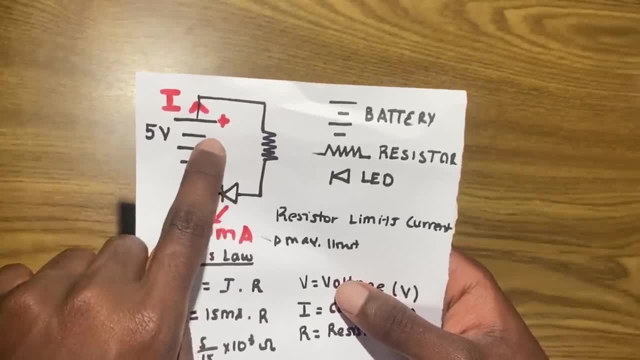 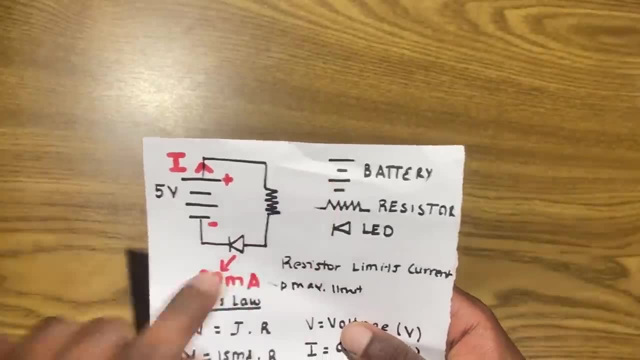 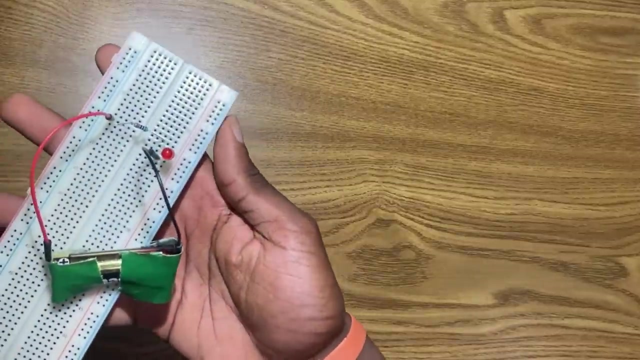 nothing more than that, something that outputs five volt. we only used it as something that outputs 5 volt but also can output a voltage- a battery can, so in this case, we can build the same exact project if we have a five-volt battery. okay, so instead of using an Arduino as a power source, we can use a. 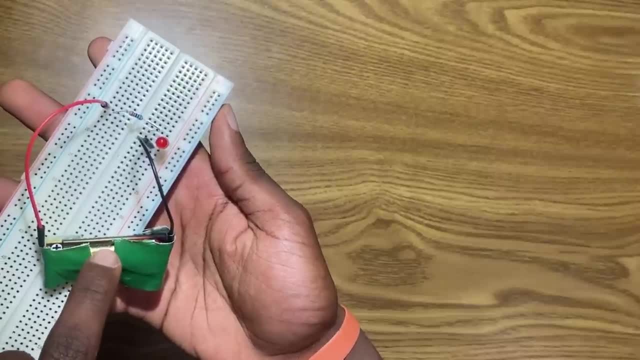 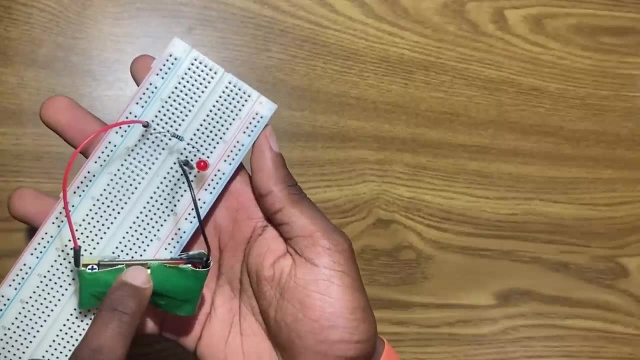 battery. right here I have a 1. volt battery, as it's just found commonly inside of, uh, the remotes and all that, all the things that we use. so i'm going to use a 1.5 volt, but this means that current is going to be less. okay, so. 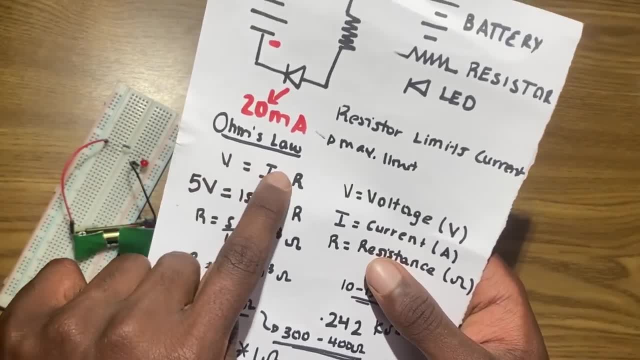 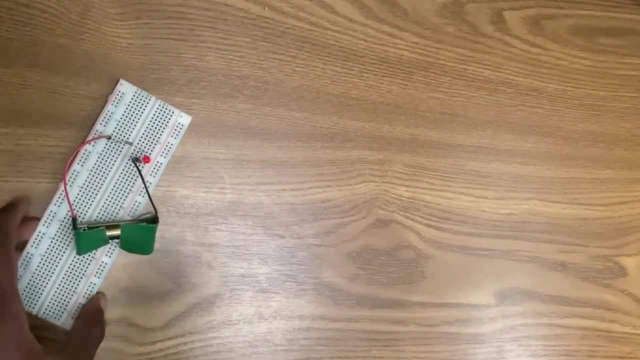 voltage is directly related to current, so i'm going to have less current. basically it's going to. the light is going to be a bit more dim. so to actually demonstrate that, let me turn off the light. maybe then you can see it. if you cannot, let me just bring this paper right here and try to. 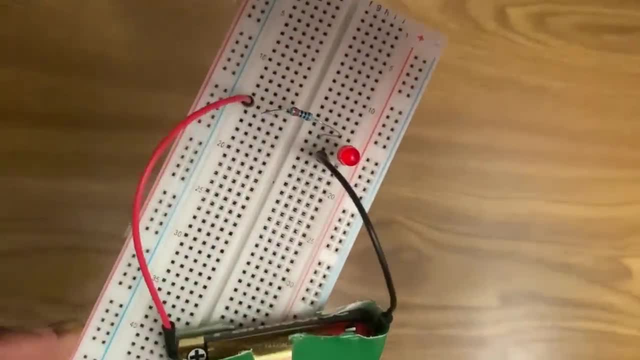 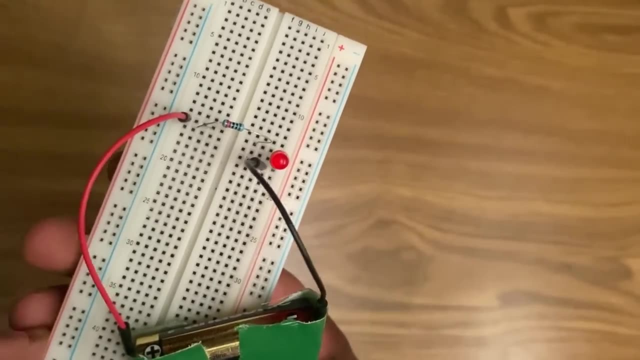 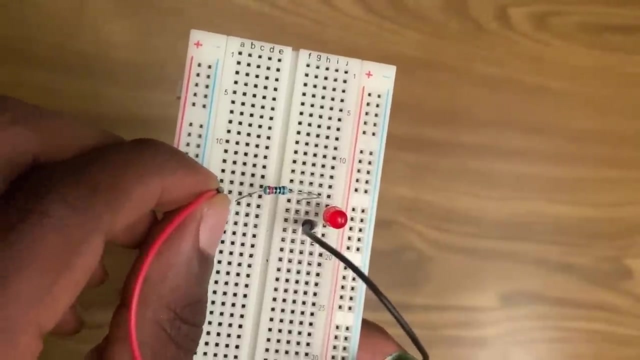 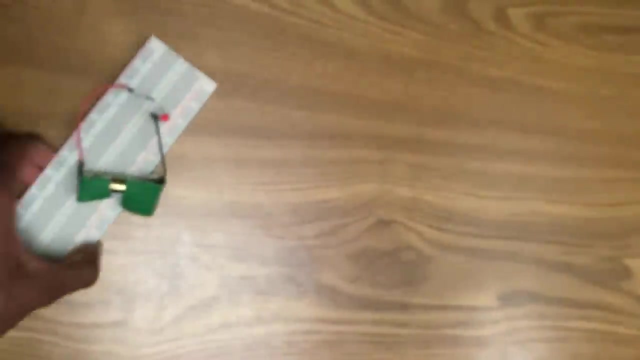 overlay it with the paper, maybe then you can see it. can you see it? okay, there we go, and let me just turn it off and turn it on so you can see the difference. you know it's it. there we go. it's very dim though you can see it. if you, it's actually in a dark environment, but anyways, this raises the. 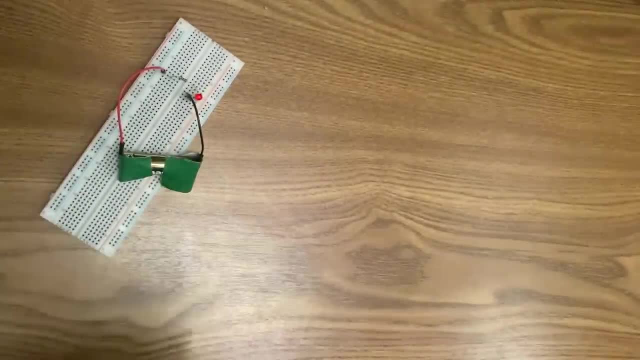 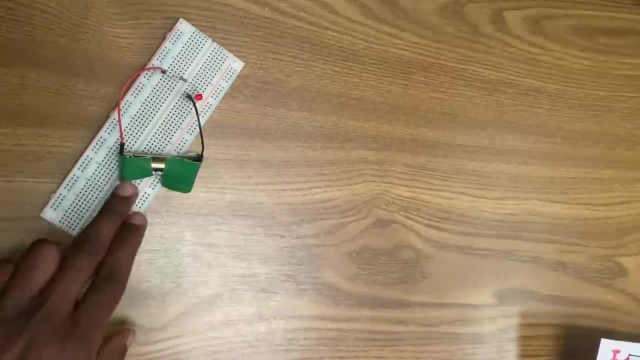 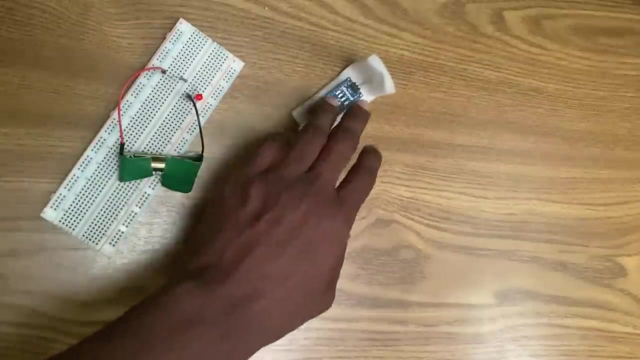 question: why not use batteries instead of arduino? because when you look at batteries, they look more reliable, they're cheaper and, again, they're easier, far easier, to just uh move from place to place, so they're more convenient. so when you, when you look at arduino right here, we have all these. 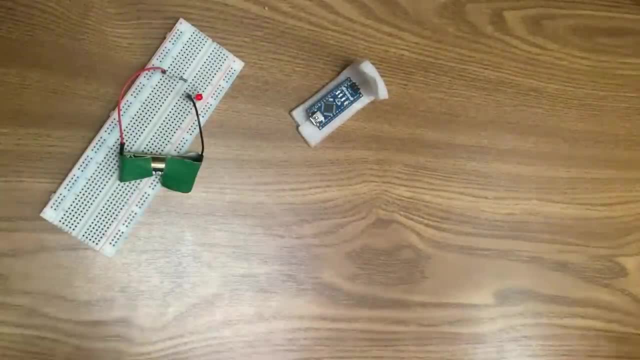 things. you really need to be careful with arduinos. not only that, too, but they're really expensive relative towards the battery. so this raises the question: why arduino? why are we using an arduino? so one thing you guys need to know about arduino is: arduino acts as a power source, but it's just. 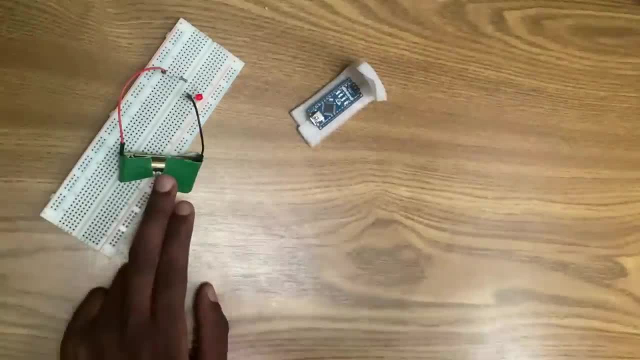 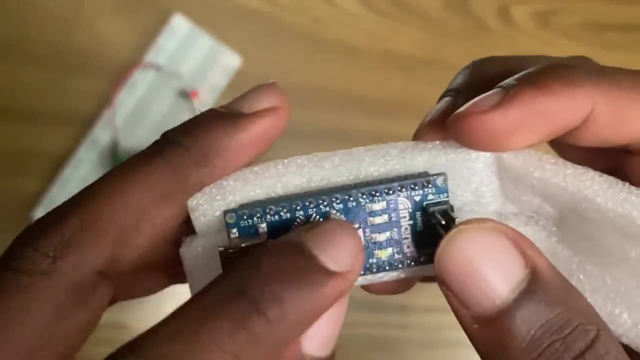 more than just a power source. all right, so it is a power source, it acts like it, but definitely it is more than just a power source. even by looking at these pins and looking at all these things that we have right here, you can see that it's just definitely more than a power source. we're only 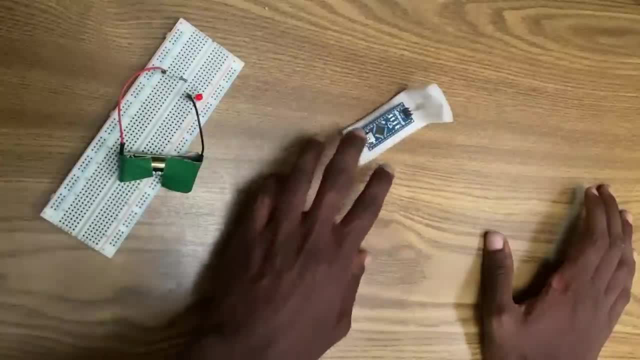 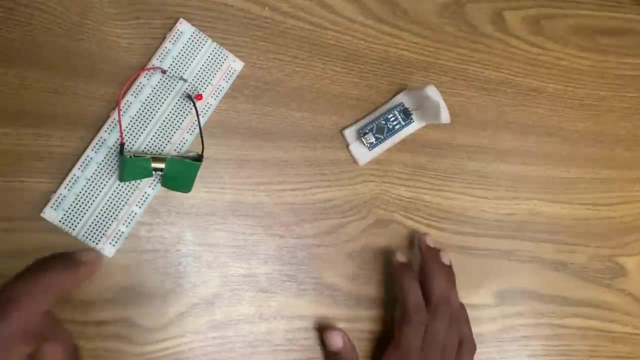 talking about the five volt right here. so when you look at all these things that we have right here, it is definitely more than a power source. so what is the purpose of an arduino? arduino is used to code our electrical components, for example. let's say i wanted to code this so that it 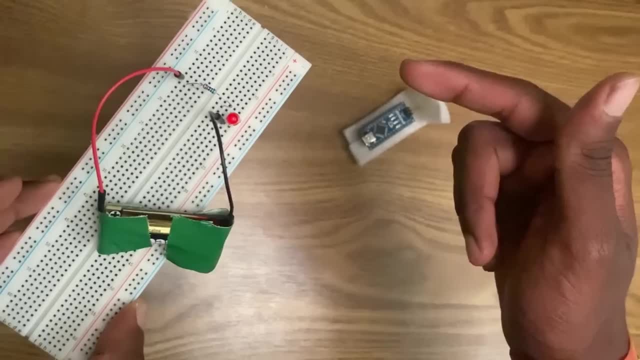 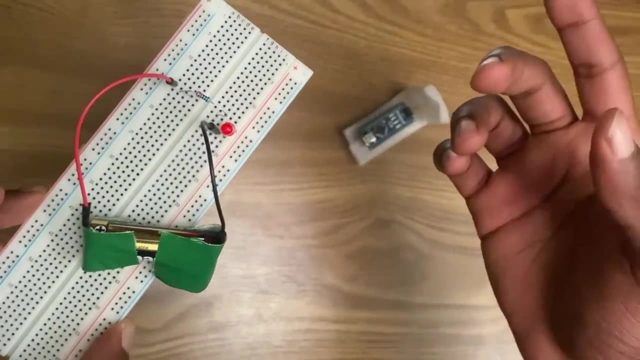 turns on and off every second, So it's gonna turn on for a second, then turn off for another second. turn on, turn off doing it in the loop. Okay, so it's gonna turn on for one second. turn off for one second. turn on for one second. 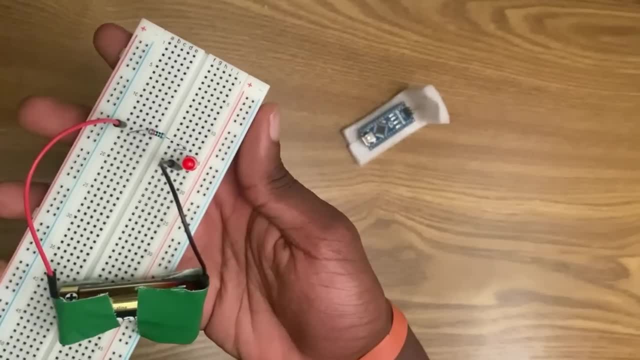 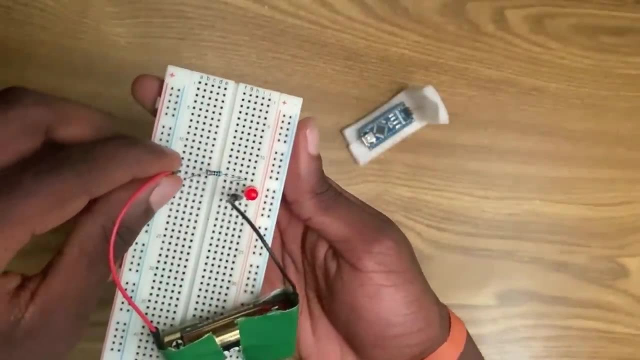 turn off for one second and keeps going on in the loop. So how do I do this? using a battery? I have to physically come in right here, turn it off, turn it on. count a second. turn it off. count a second, turn it on. 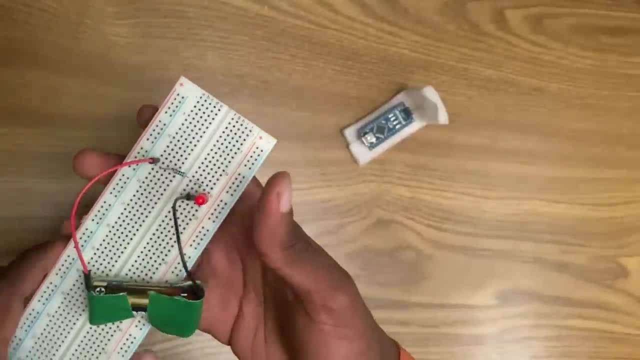 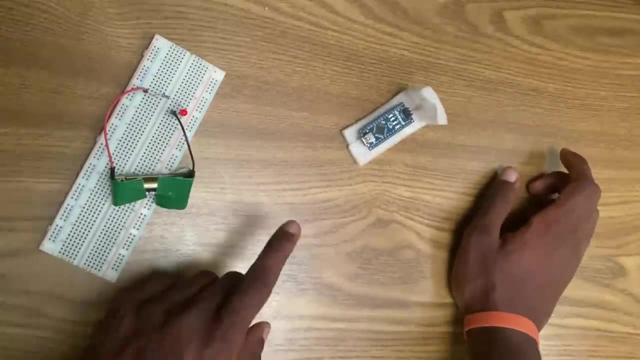 count a second, turn it off, And obviously this is not coding, But with an Arduino we can set this up, We can set up, we can set this up so that we can actually code it to actually make it blink. So we're gonna turn it on for one second. 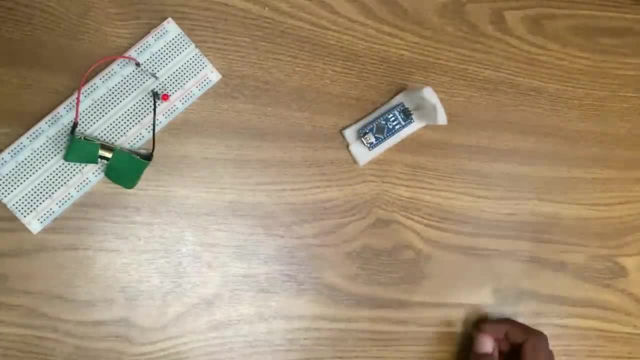 turn it off for one second. We can do this using an Arduino. So Arduino, what does it do? Something important that it does is: lets us code our physical components. I'm sure you use websites and applications and they're coded digitally. 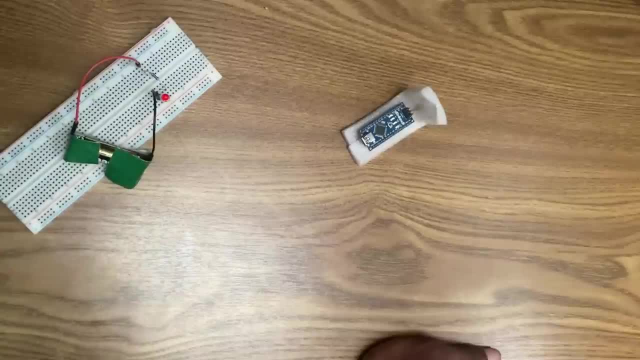 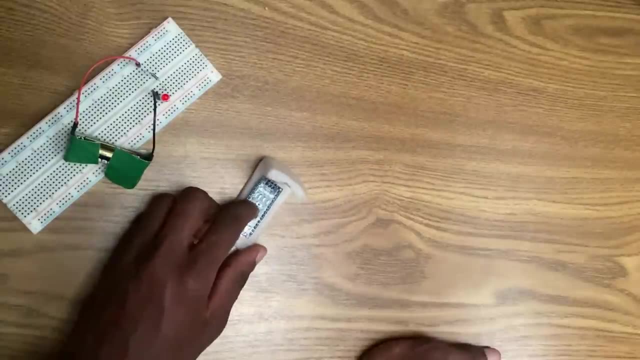 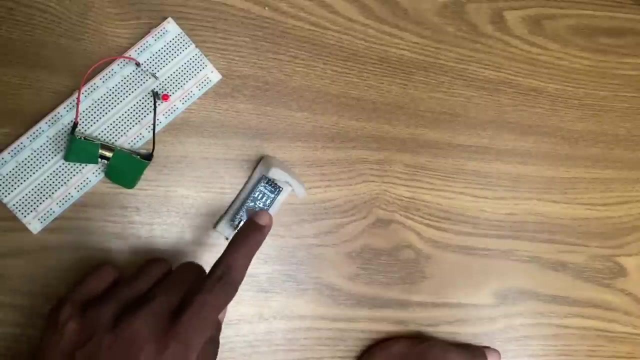 So what if you wanted to code our physical components, For example? let's say we're working on a robot or some other projects. This is where Arduino comes in. This is where Arduino comes in and lets us code our physical components. So definitely, Arduino acts as a power source. 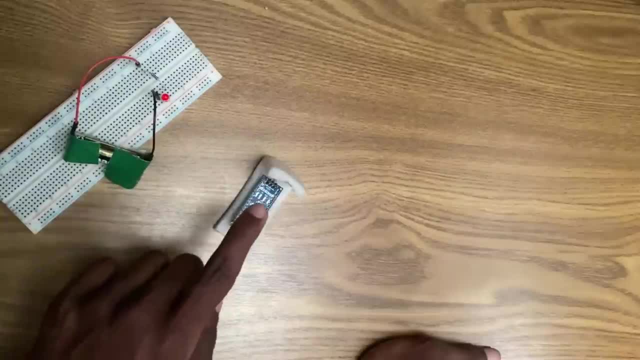 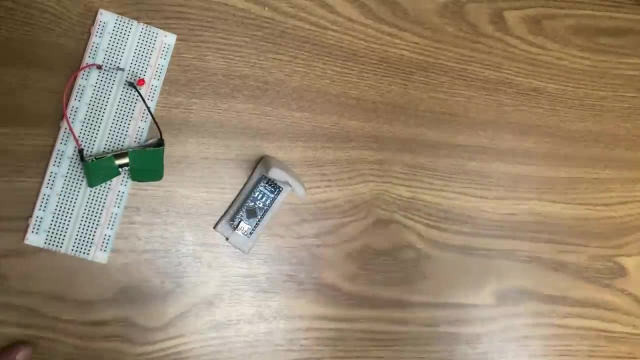 but it acts as an intelligent power source. all right, An intelligent power source that we can code. okay, So it's definitely more than just a power source. All right, with that in mind, let's check how to actually code our Arduino. 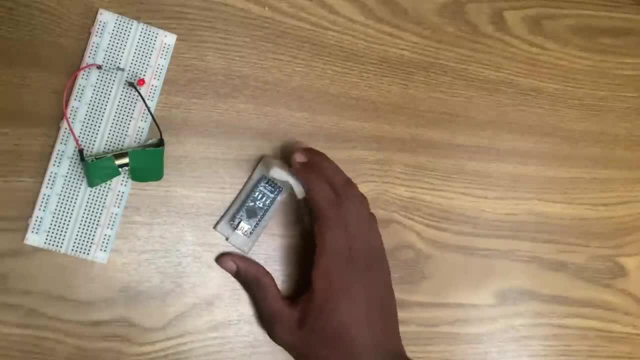 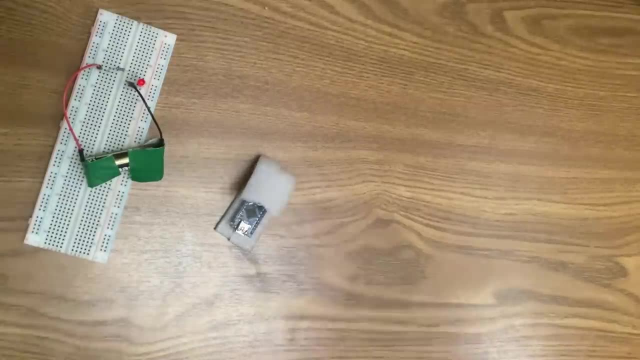 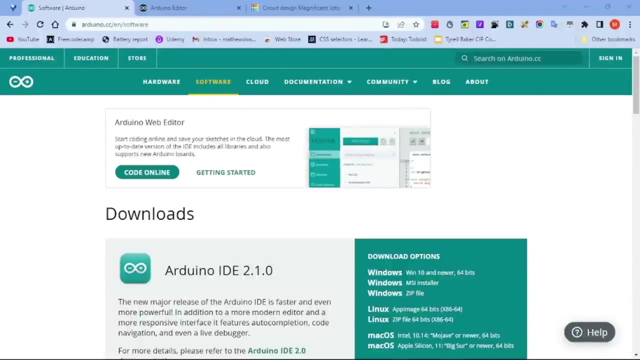 So how to actually put transfer code to Arduino. So see you in the next section, where you're on my screen and we actually check on how to code using an Arduino. So far, we've learned that Arduino is more than just a power source. 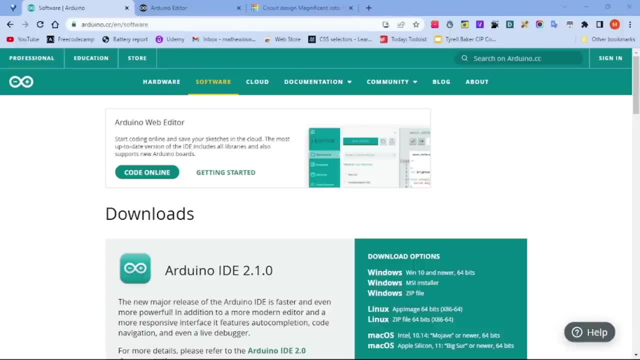 and it can do a lot more, especially letting us code our electrical components. So to start coding our Arduino like a controller, we're gonna need a platform to write code on, So in this case, we're gonna need a code editor. So it's gonna be different. 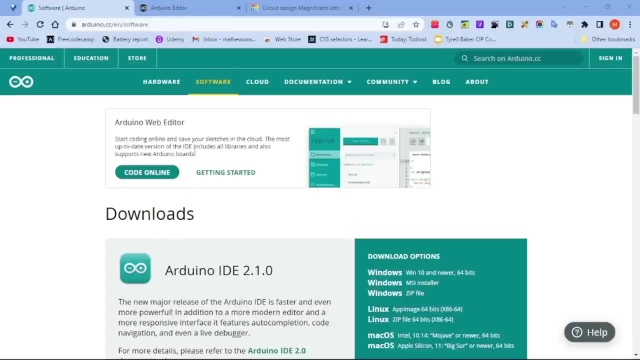 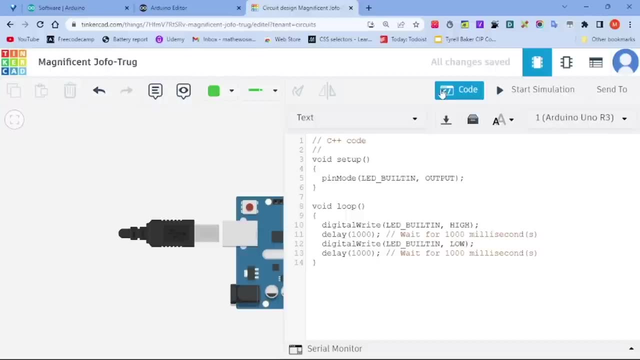 depending that you're gonna be using a physical Arduino or additional Arduino on a simulator. For those of you who are using additional Arduino on a simulator, all you need to do is go to this code right here, this code section right here, and choose your preference. 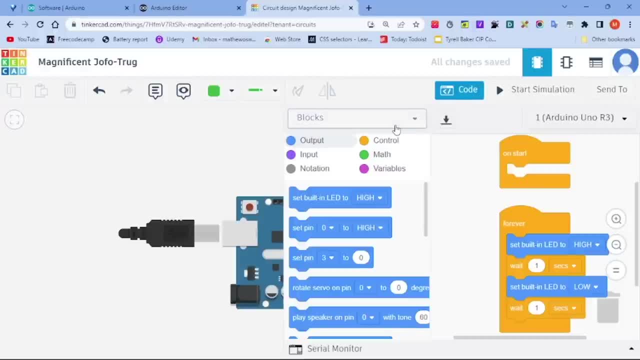 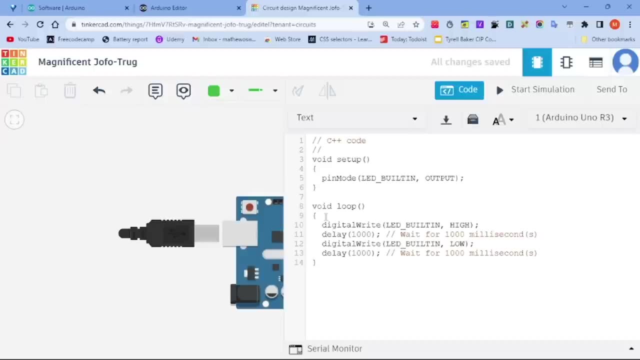 So if you're using blocks, you can use blocks right here. You can change it to block, or if you prefer text, you can use text right here, But I highly suggest that you guys use text, as I'm gonna be using text for this course. 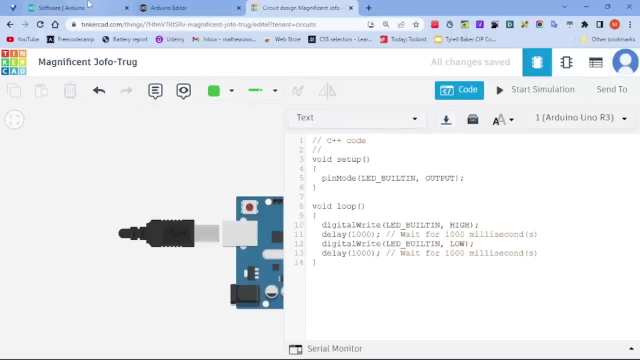 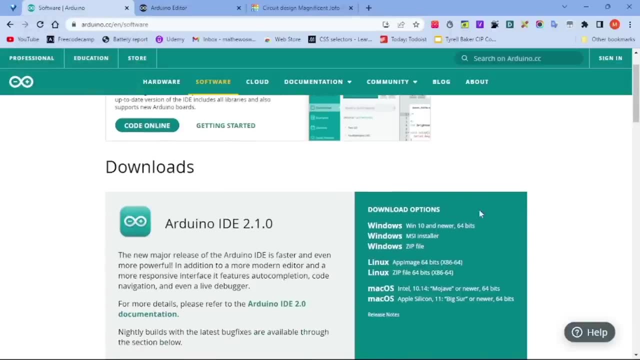 Okay. So for those of you who have a physical Arduino, all you need to do again is go right here, follow this link and download the Arduino, depending on the operating software that you have right here. So if you have a Windows, you're gonna download from here. 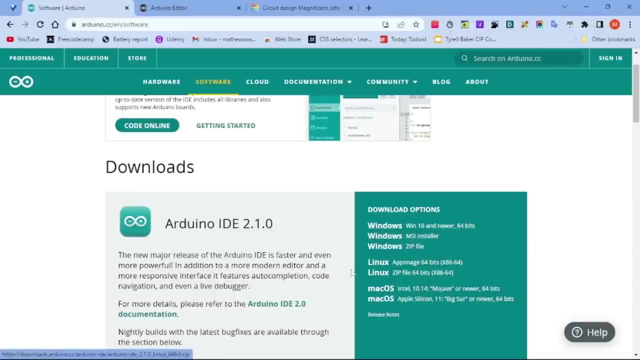 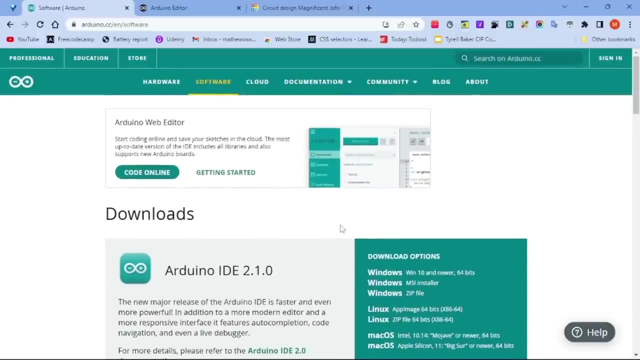 If you have a Linux from here and a Mac, you're gonna download from here. So for those of you who don't have a Linux, Mac or Windows- or maybe, for example, you're using a Chromebook- all you can do is go to your Arduino web editor. 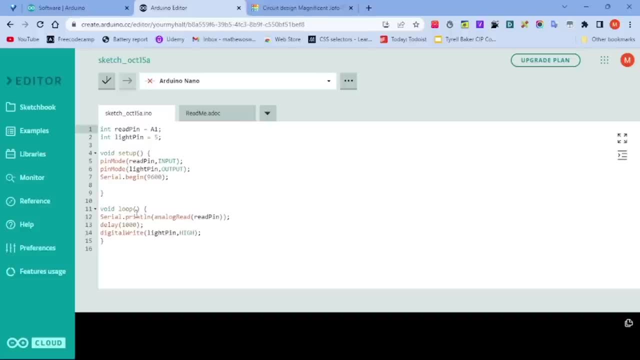 and touch the code online and sign up and you can use this Arduino web editor and you can use this Arduino web editor and you can use this Arduino web editor. so, without downloading anything, you guys can just start coding to your Arduino. 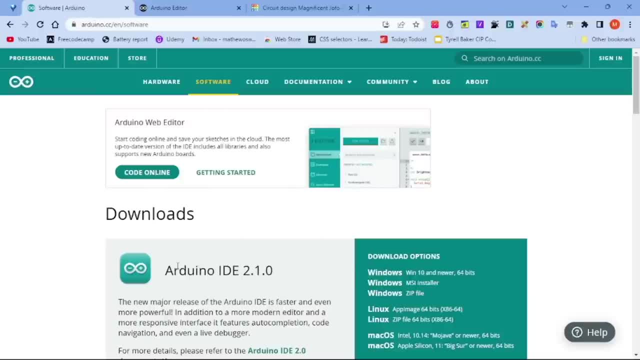 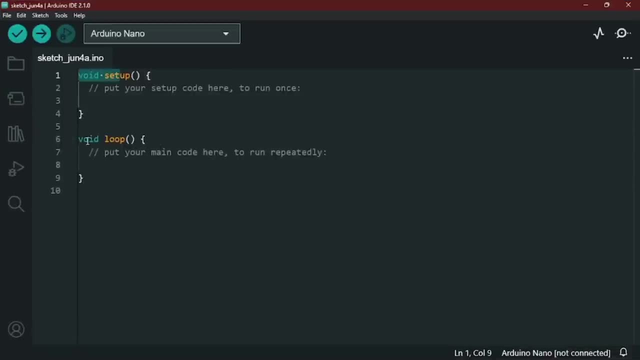 That's all you need to do. start writing code to your Arduino. So once you're done downloading the Arduino code editor, it looks something like this. There we go. It looks something like this: It has void setup and void loop. We're gonna check what this means. 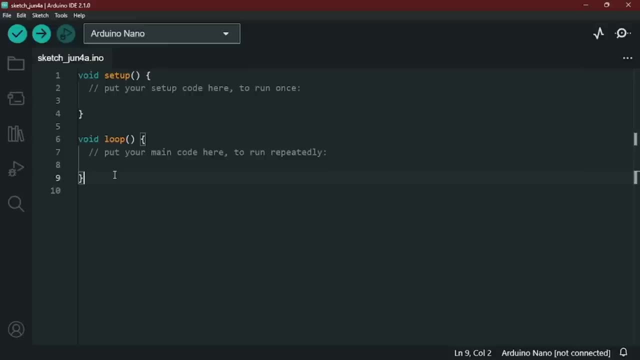 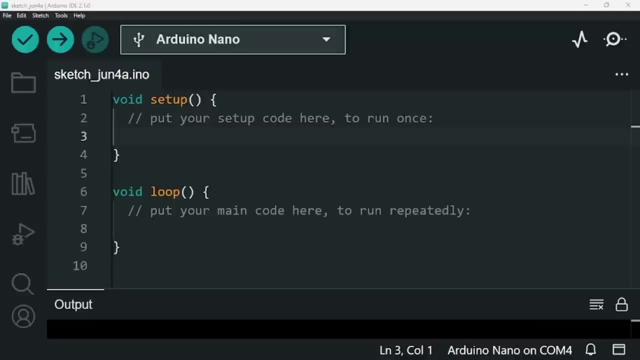 and not only that, too, but we're also gonna create this Blink project that I mentioned earlier of the LED earlier in the next section. Okay, So now what do we wanna do to write code to our Arduino? Let me go to our code editor. 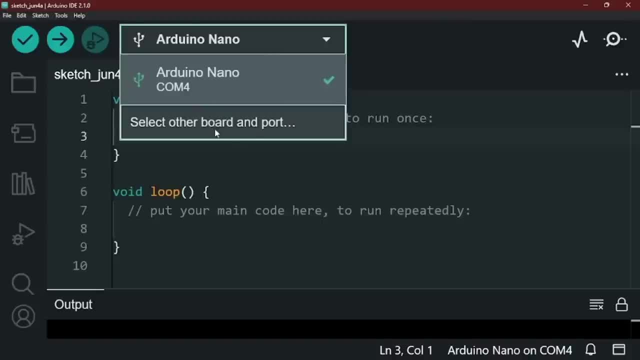 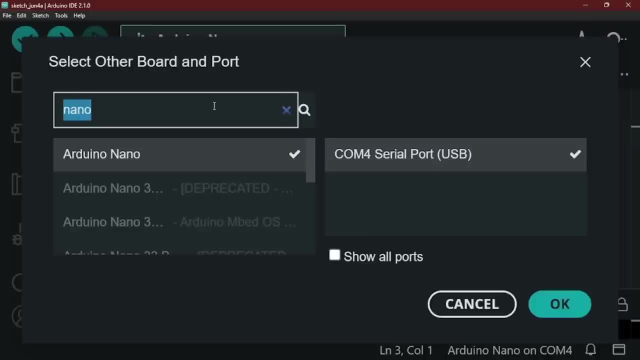 and one thing you need to set up is go to our Arduino and choose our board and our communication port. okay, How do we do it? We go and select the board that we're using. For example, let's say I'm using an Arduino Uno. 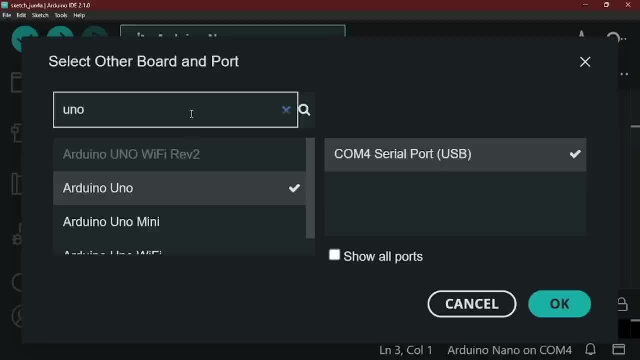 I go to Arduino Uno and select it. Obviously, I'm using an Arduino Nano, so I'm gonna go back to Arduino Nano and select it, So you're gonna choose the Arduino board that you have right here Once you're done with that. 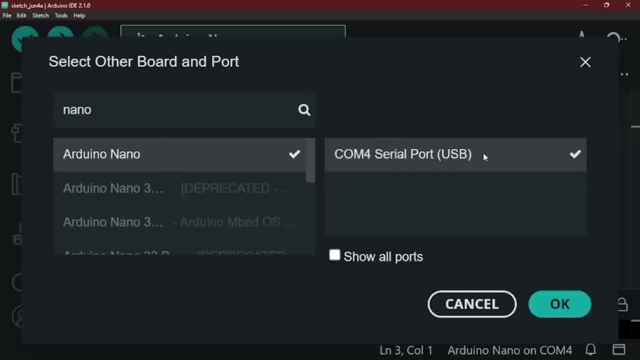 you're gonna check the communication port that you wanna use Right here. I only have one communication port, so I only have one COM port. So I don't have to stress and I can just continue and just say, okay, But let's say we have two, maybe two communication ports. 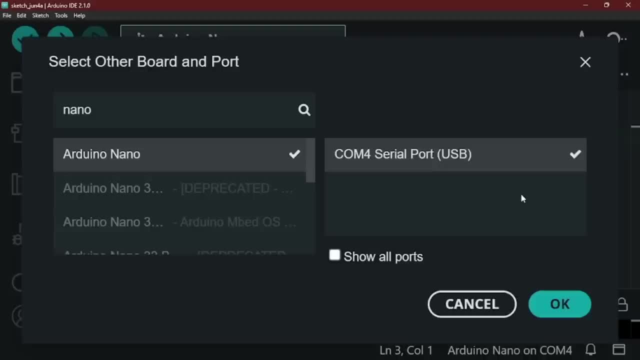 Let's say, I have another communication port right here underneath and you do not know which one to use. To know which one to use, all you need to do is basically plug off your Arduino. So I'm gonna plug it off, and once I plug it off, 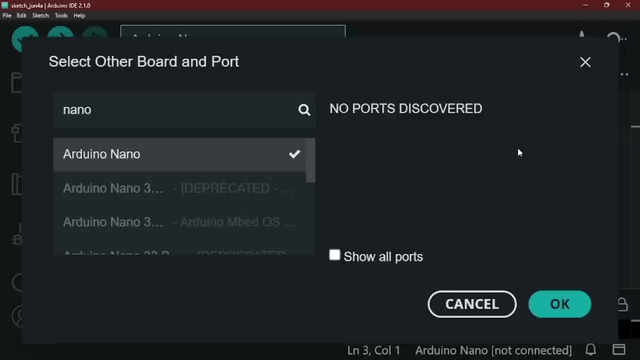 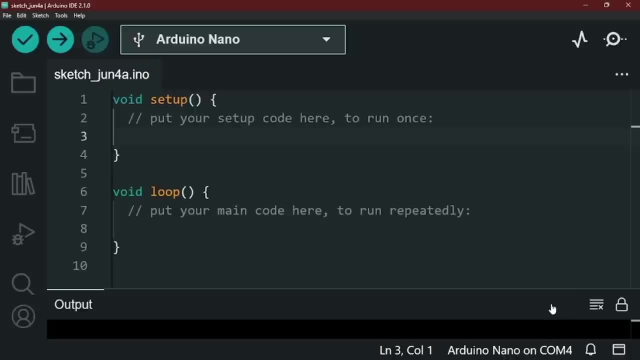 it's gonna turn off. The communication port is gonna be off, So you're gonna know which communication port is tied to your Arduino. Okay, there we go. Go back to touch. okay, Then I'm gonna need to write code. So this is a starter code. 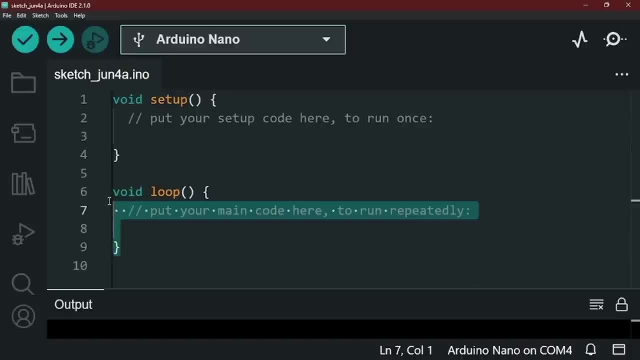 This is a code that always exists for every sketch. Okay, so this is gonna be a code from the complex ones, The easiest project. they're gonna contain void setup and a void loop. Okay, so what is a void setup? This is where we actually put our setup code. 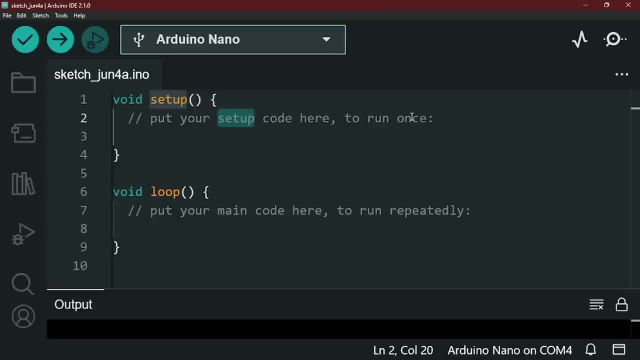 Okay, and it's gonna run once. Importantly, it's gonna run once Okay. so we're gonna put our setup code right here and we're gonna only write once Okay, when it comes to loop, we're gonna put most of our code. 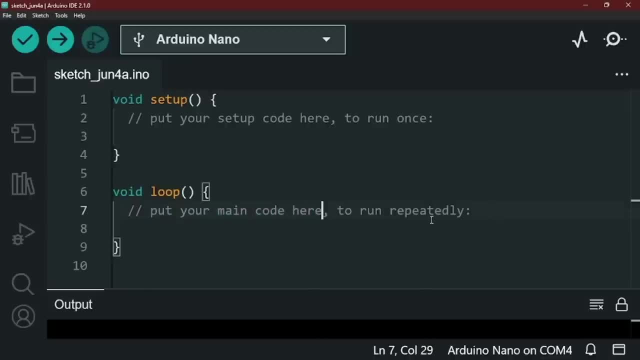 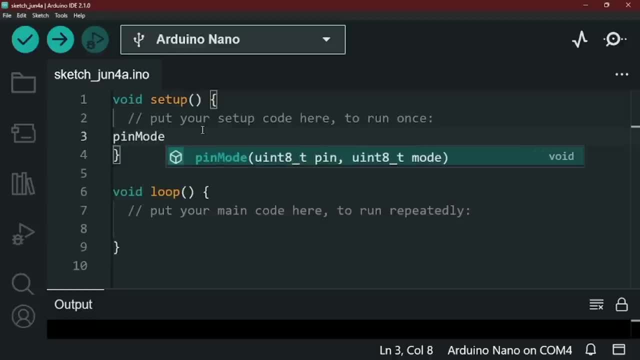 we're gonna use this built-in function called pin mode. Okay, we're gonna use something called pin mode. All right, there we go And we're gonna tell it what pin we wanna use. Right, here I have again from two to 13.. 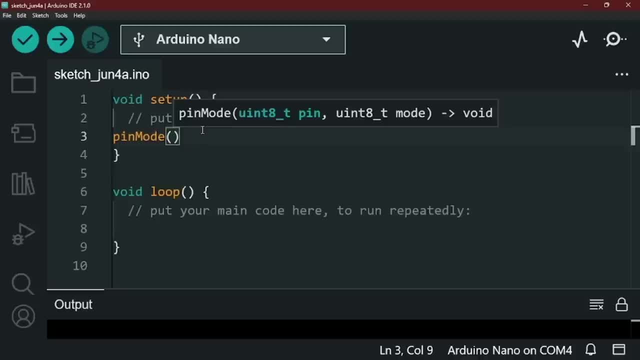 I have digital pin two to 13.. So I'm just gonna choose random number. Let me just choose seven for now. So we're gonna use pin seven. Okay, then, once we're done letting our Arduino know. Okay, then, once we're done letting our Arduino know. 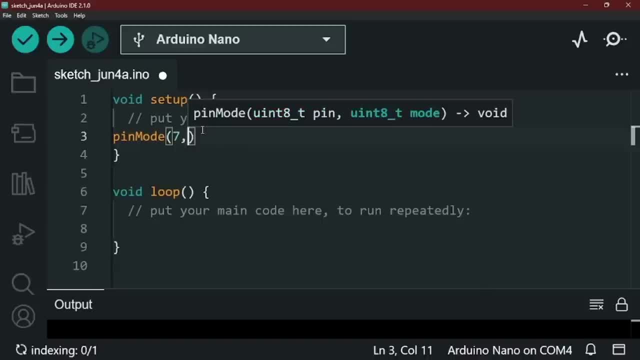 Okay, then, once we're done letting our Arduino know which pin we're gonna be using, we're gonna notify it of how we're gonna use it. okay, So we're gonna tell it if we're gonna use it as an input or we're gonna use it as an output. okay. 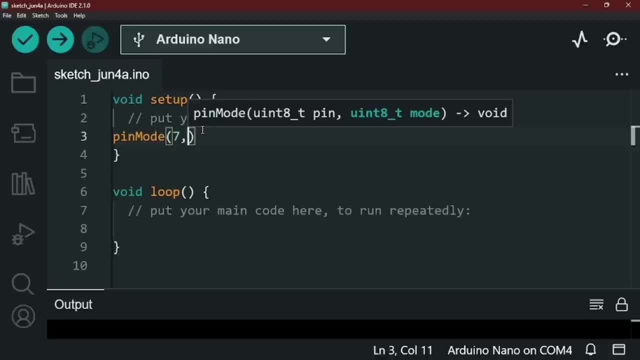 So if you wanna use it as an input, you want to what? You want to receive data from the pin- okay. So when you wanna use it as an output, what do you wanna do? We basically want to send data. In this case, we're gonna send what? 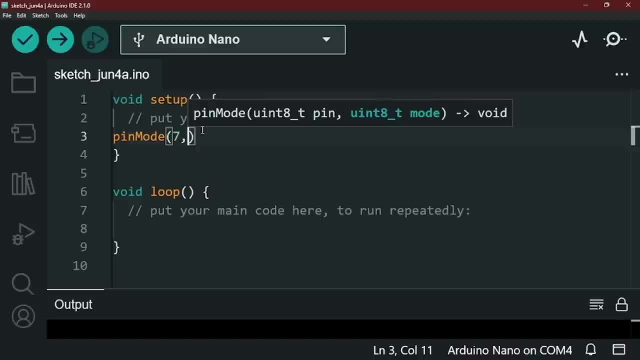 Electricity. okay, We're gonna send voltage okay, So we wanna use it as an output in this case. Once we're done with that for every line, when we finish a code for every line, we're gonna finish it with a semicolon, okay. 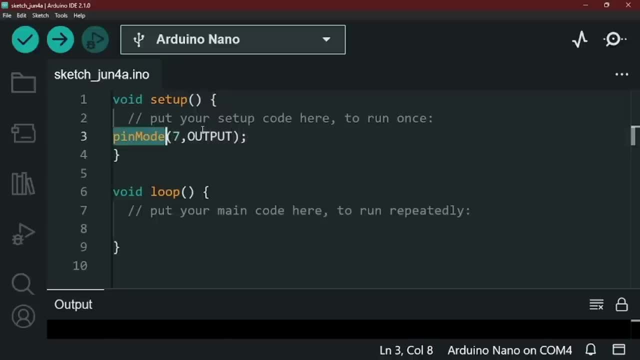 So one thing to keep in mind is for all of you is capitalization does matter, So you cannot write down pin mode, let's say with a small m. If I did that, and let's say I wanna verify the code. 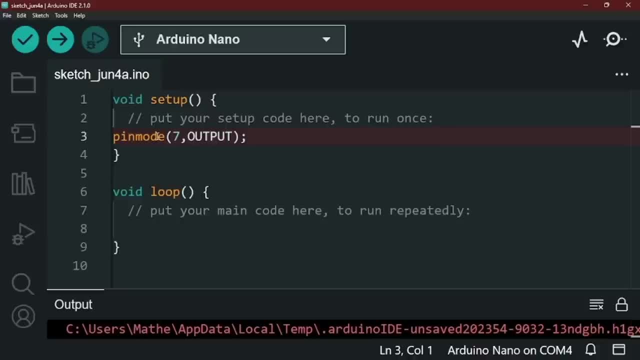 it's gonna show me an error message. So one thing you wanna keep in mind is: every time capitalization matters in code, okay, So it even matters for this output. Let's say I see output right here with no capitalization, with no proper capitalization. 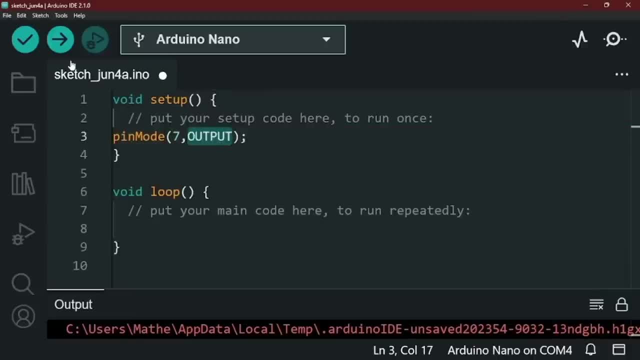 it's gonna give me an error, okay, So capitalization is very important in coding, And let me just run this right now. I don't see any error. Okay, there we go. So I wrote this down properly. So what does this code do? 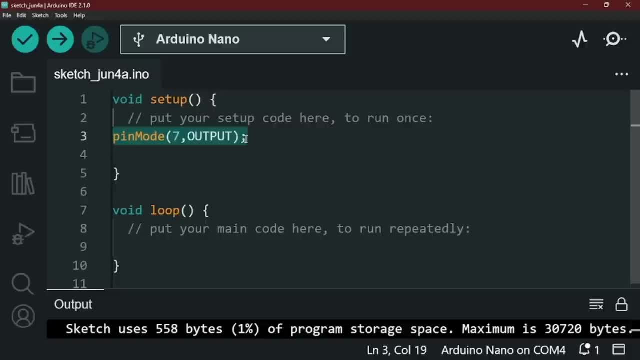 It tells our Arduino that we're gonna use pin seven. How do you wanna use it? You wanna use it as an output. So once we're done notifying our Arduino and we're done setting up our pin, okay, We're gonna go to our loop, okay. 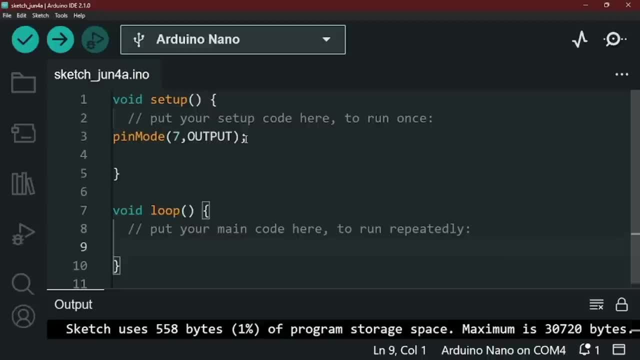 So how do we tell Arduino if you wanna give five volt and zero volt? we're gonna use something called digital write. So right here too, again, specifically, capitalization is very important. So what pin do we wanna write? We wanna write down pin seven. 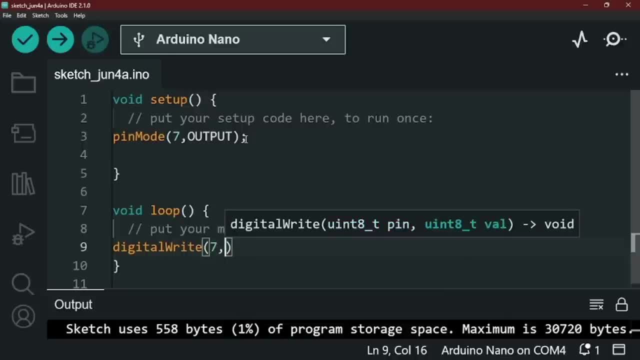 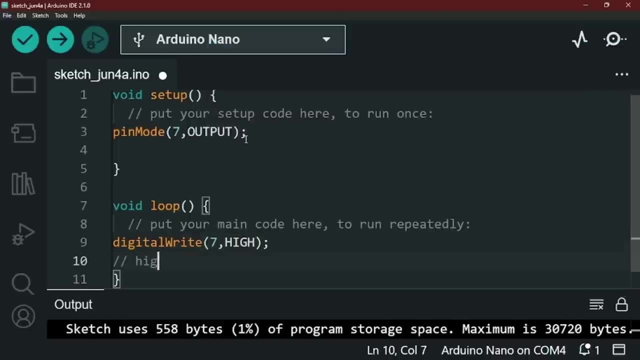 that we already set up right here. There we go, And once we're done with that, you wanna tell it if it's gonna be high or low. High basically means, basically. high means five volt. okay, High means five volt, five volt right. 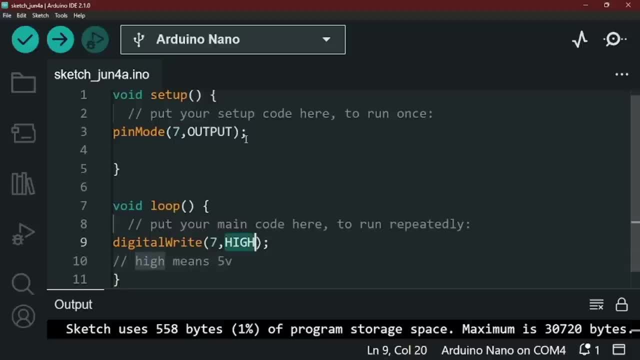 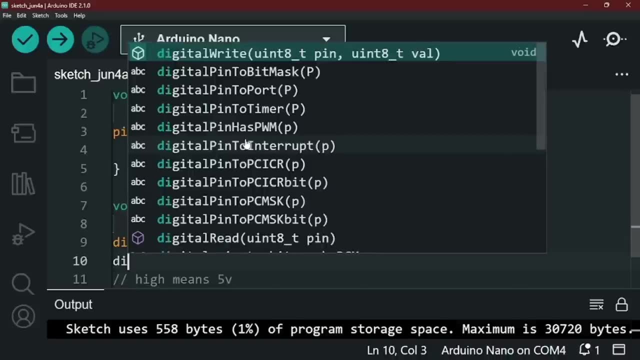 You wanna keep this in mind. So high? this basically means what? Five volt. Okay, then, once we're done with that, what do we wanna do when we wanna make it blink? We wanna what. We wanna write down the same code right here. 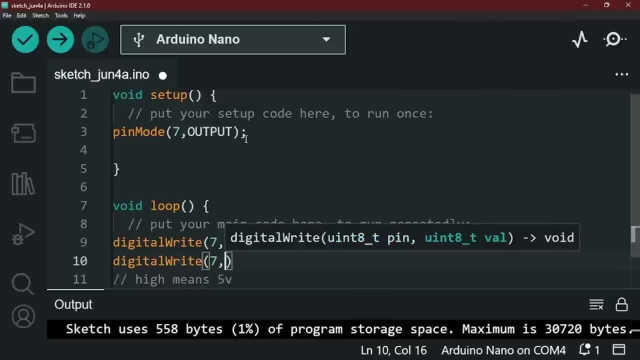 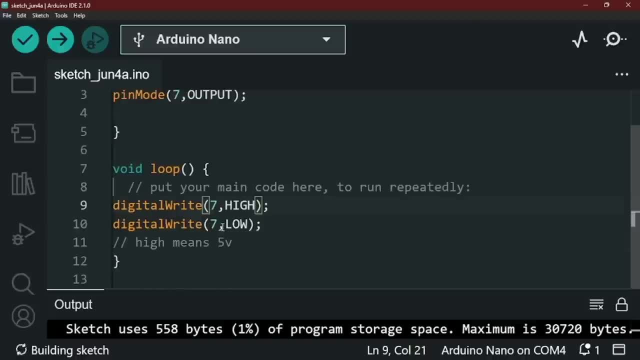 Again, capitalization matters- And put pin seven- and you've guessed by now: we're gonna use low, We're gonna use low. So what is it gonna do? We're done setting up our code once, so we're gonna notify Arduino what pin we're using. 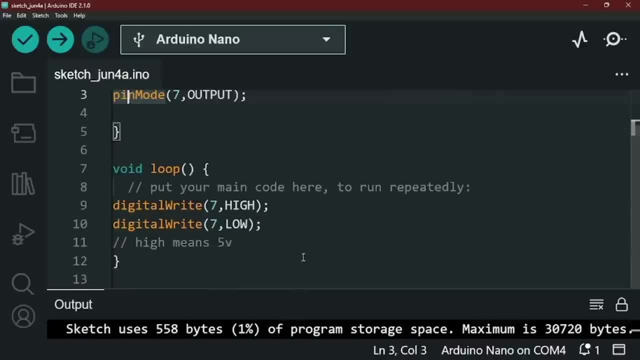 and how we're gonna be using it. And once we're done with that, it's gonna run this code as a loop. It's gonna run it repeatedly right here, okay, So it's gonna go pin seven. it's gonna turn it high. 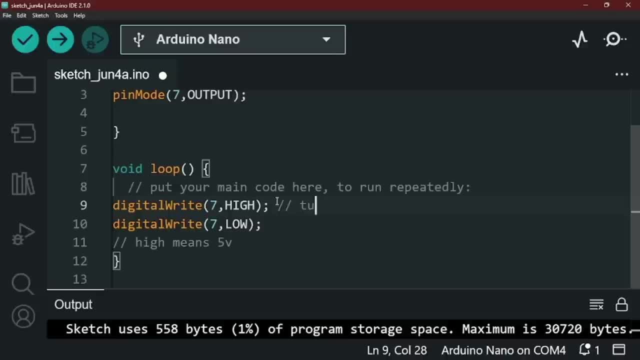 It's gonna turn it to what? To five volt right here. Turn to five volt And then, when we turn it to low, we basically turn it to zero volt or off. Five volt or on. okay, That's what we're gonna do. 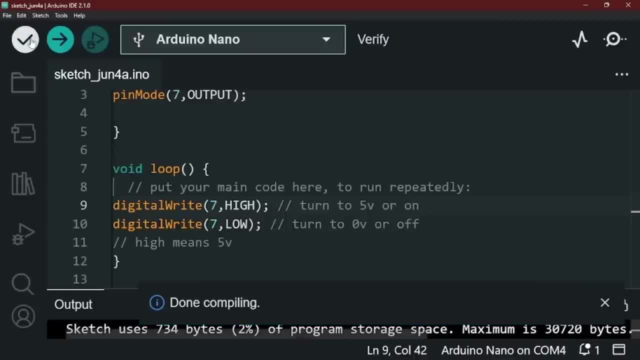 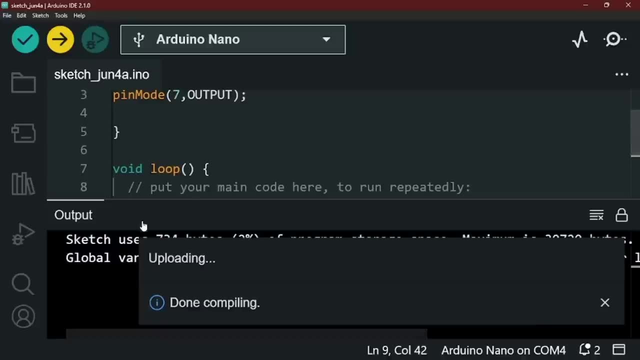 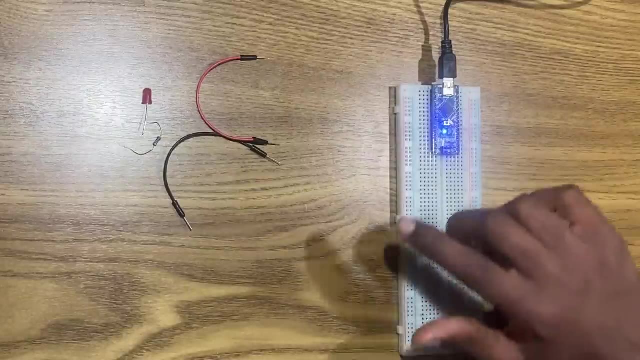 So let me just do is verify the code right here in case we have an error. It's done compiling right here properly, And then what we do is upload it. okay, And we're gonna upload it to our Arduino. But one thing I forgot to do is to set up our Arduino. 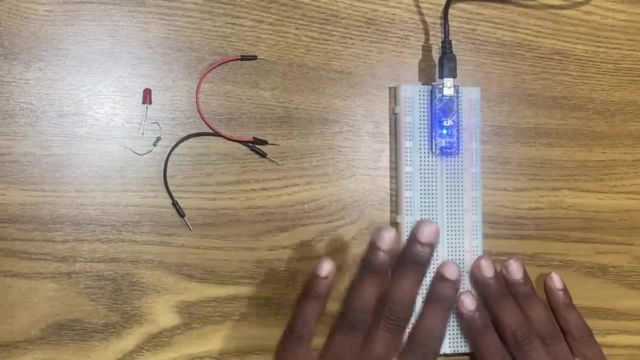 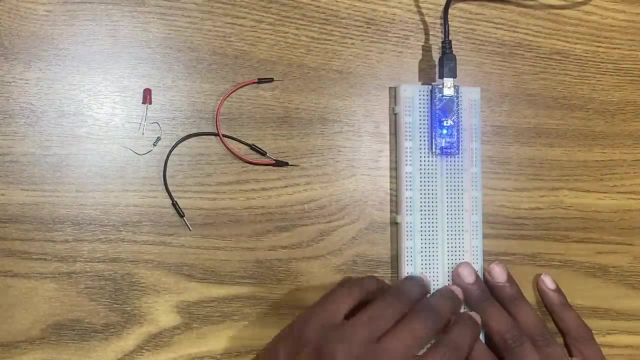 So we need to set up our Arduino. So one thing I need to do right here, before even setting it up and wiring it, as I told you guys before in the precaution, safety section, what I told you guys was to turn off our Arduino. 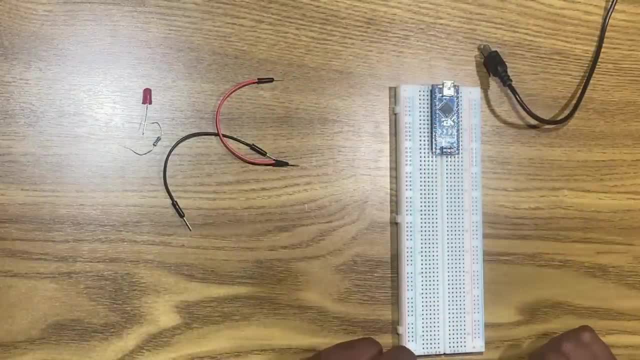 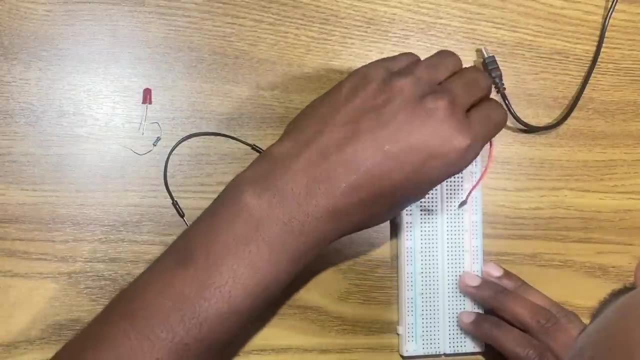 First we build our circuit and then we turn it on. okay, Okay. so let me bring my red pin right here and attach it to pin seven. Wait, that's pin two. Pin seven is right here. Okay, there we go. 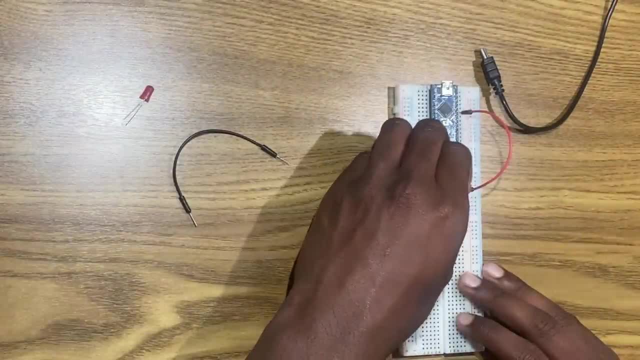 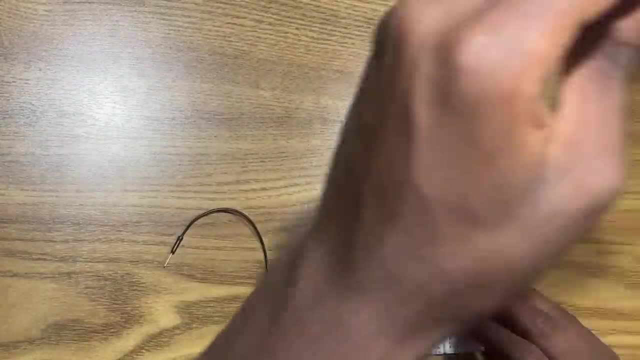 Put it right here. Put our handy resistor right here. We wanna put it at an intersection. There we go. Okay, then we need our LED. I'm gonna need to know. the big side is obviously the positive. There we go And put that right here. 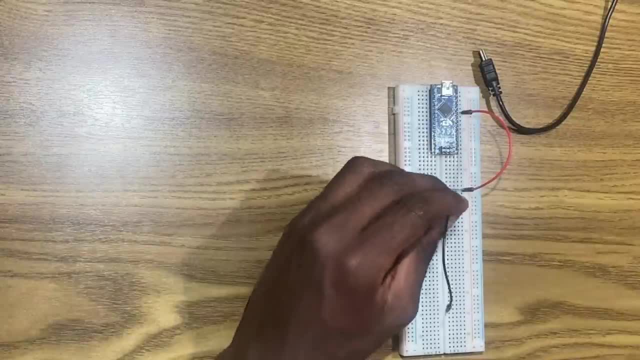 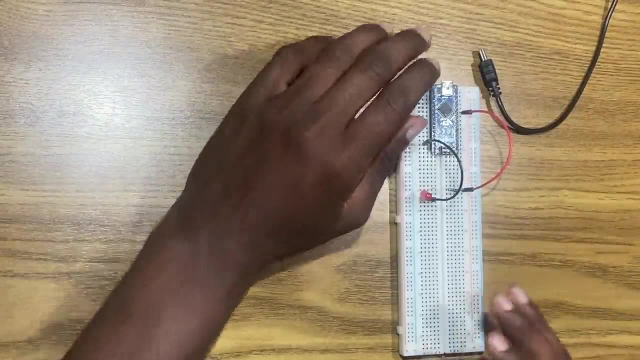 the positive with the positive side, And then we're gonna go back to our GND or negative terminal. Let me go to GND right here. There we go. So I wanna check again up close if I'm actually correct or I'm making mistakes right here. 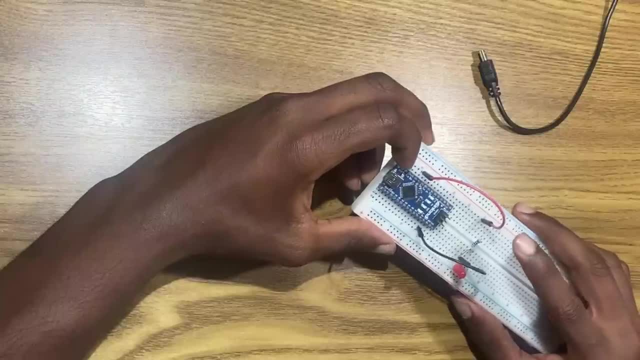 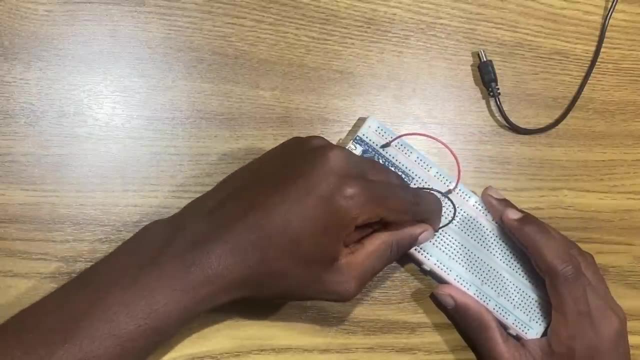 So I'm just gonna bring it closer to myself and check it for myself. Okay, that seems fine, Nice. okay, let me check the wrong side again. Okay, there we go. I'm correct. All right, I'm done checking. 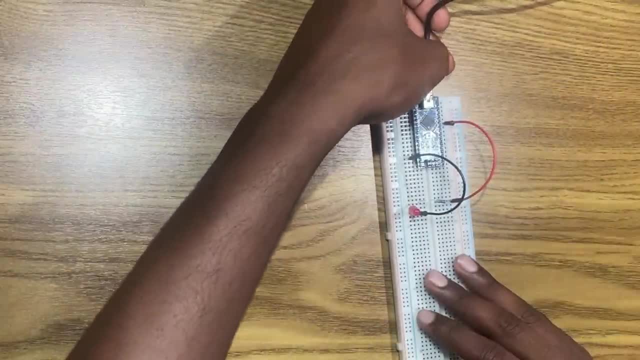 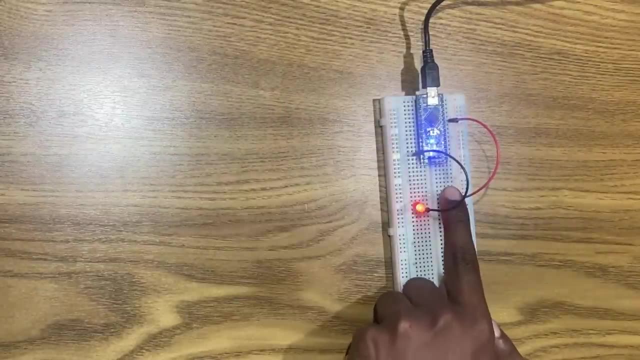 Now I can turn on my Arduino. Let me turn it on. Okay, I think it's the resistor right here. Okay, it was the resistor, so let me just touch it again. Okay, there we go. it's working now. 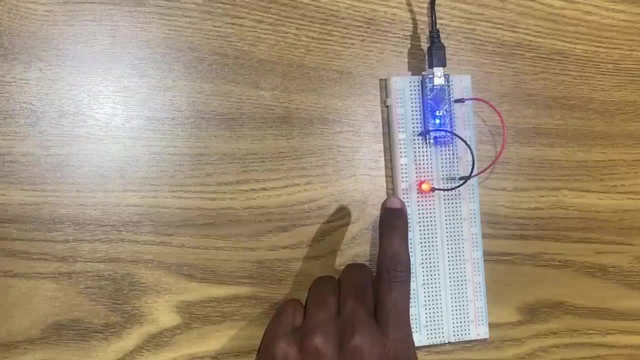 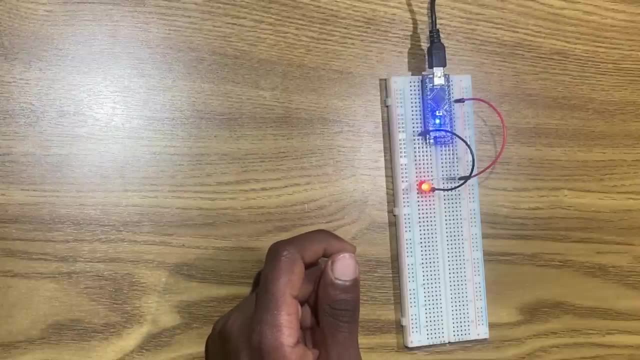 But can you with something? it's not turning on, it's turning off, It's just not blinking. We cannot see any blinking right here. can you? I cannot, So what is happening? So let's analyze our code. So what we did was set up our code. 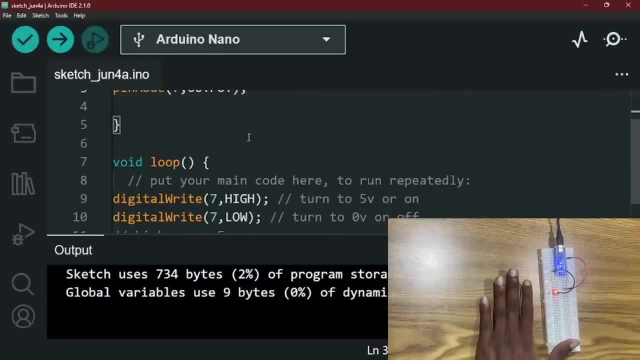 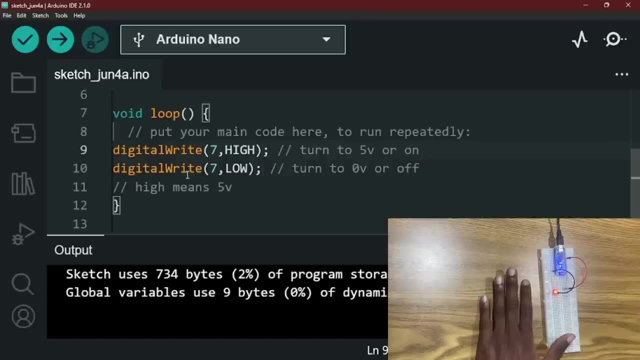 Everything seems fine, right here, Everything seems appropriate, And then what happens is basically what happens is we digit the right and we set it to high, then we set it to low, then we set it to high and low, And one thing you notice is it's gonna go. 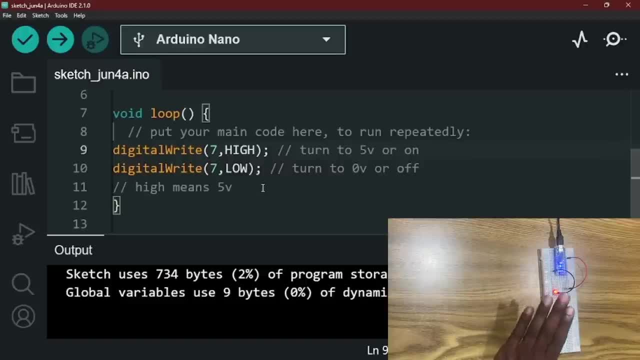 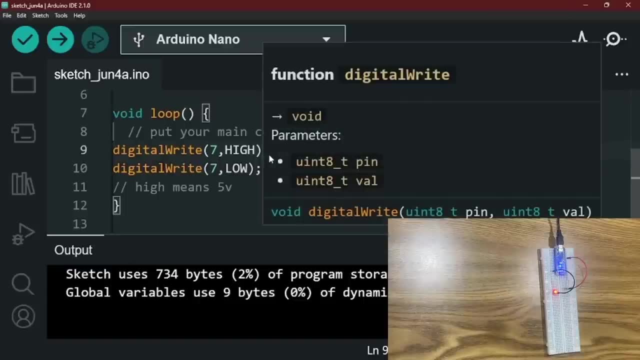 at a very fast speed. It's gonna be really really fast. Computers are really really fast, So we cannot notice this with our naked eye. So right here, look at it. It's gonna go high, then it's gonna go low really fast. 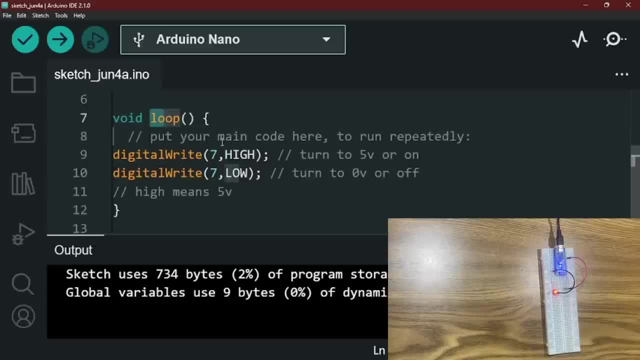 Then it's gonna go high again, It's gonna again go on a loop, as I said again. So it's gonna go high, low, high, low, very, very fast that we cannot notice it. So what do we need? 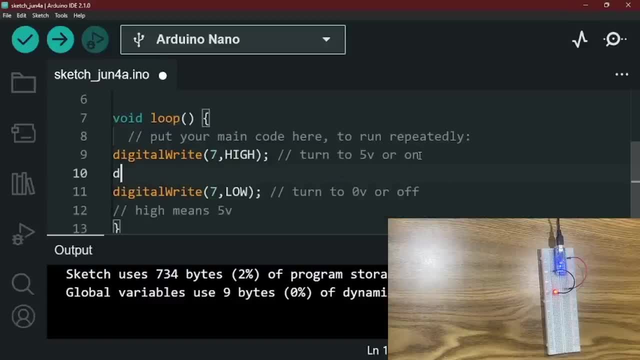 We need a delay so we can notice it, So we're gonna need a delay. So to do that, we're gonna use this delay function, okay? So when I say 1,000, that's gonna be one second, So it's gonna capture it in milliseconds, okay. 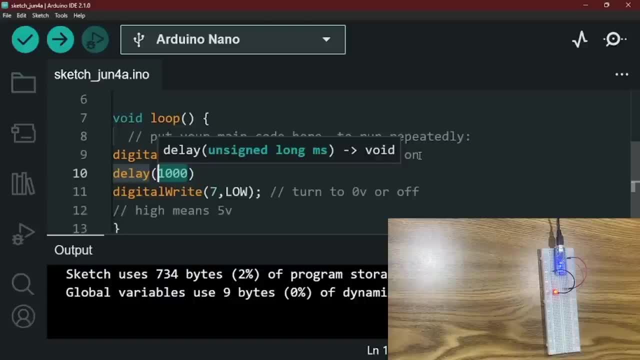 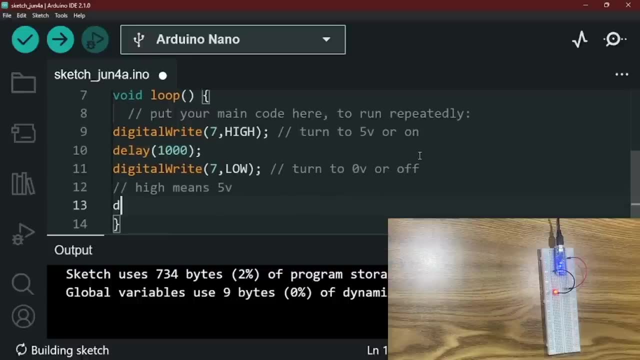 So we're gonna write down how much seconds that you're gonna delay it in milliseconds. So we wanna delay it right here and put our semicolon after every line. There we go, And we wanna put the delay right here again: delay 1,000,. then there we go with our semicolon. 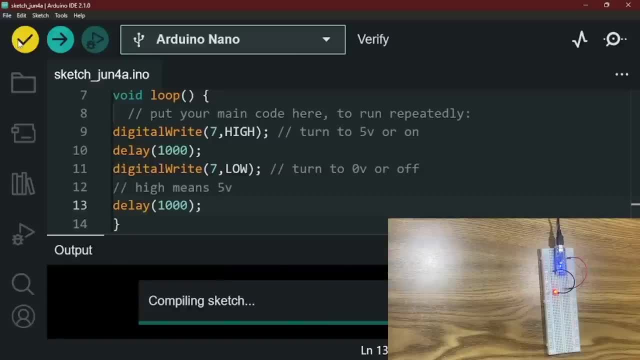 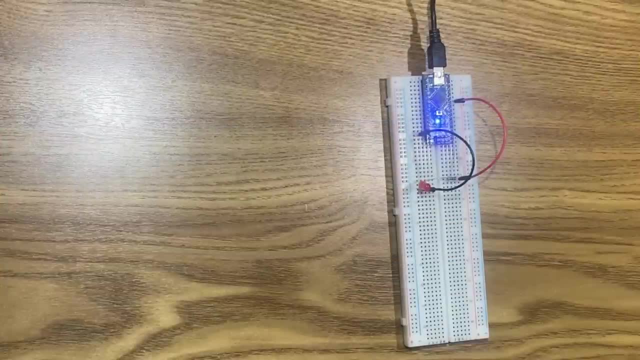 And let's run it again. So let me just verify it right now. Okay, then I'm gonna upload it. So it's gonna turn off for one second and turn on for one second, Turn off for one, on, off, on, and it keeps going on. 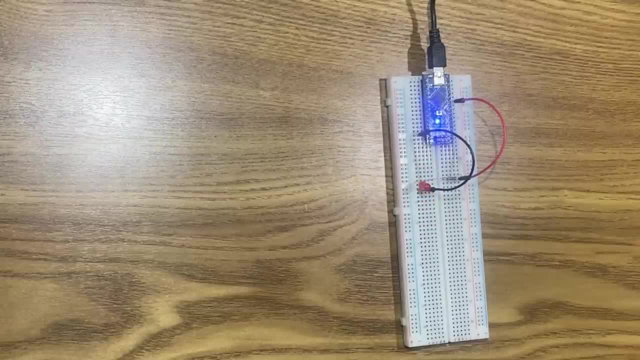 So let me go on, off, on off. So we basically build this okay. So one thing to keep in mind again is that we use milliseconds. So when I say 1,000 milliseconds, it basically means a second. 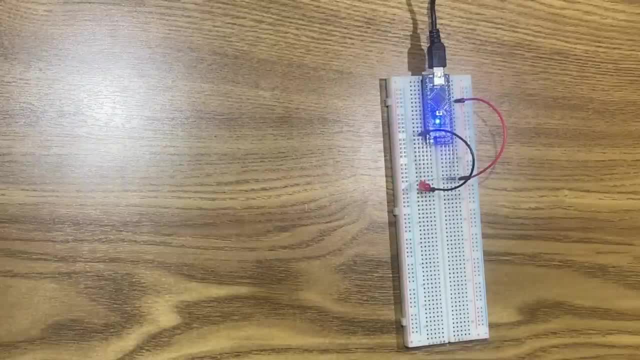 So it's gonna receive in milliseconds. Okay, there we go, So we're done. we're actually building this. So actually in the next one we're gonna check. so in the next section we're actually gonna check a few things about variables. 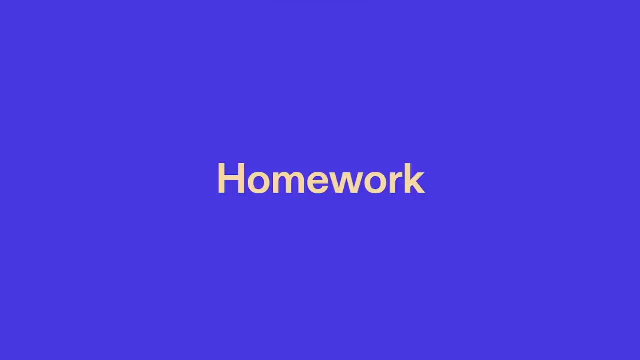 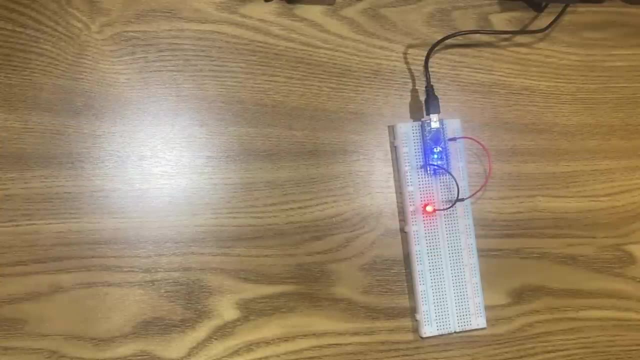 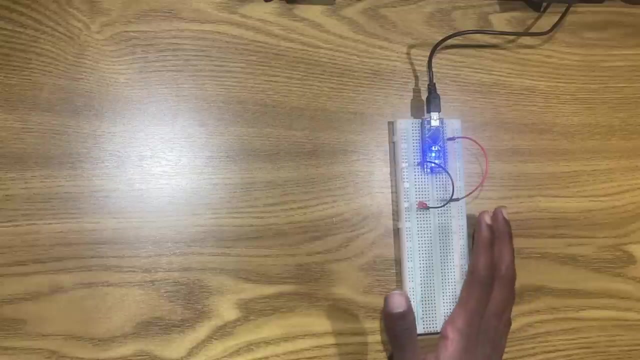 Okay, so I have homework for you guys. So, before moving on to the next sections, we're actually gonna do these homeworks, Okay. so what we did right now is obviously create this blink again. So we used one pin and create this blink. 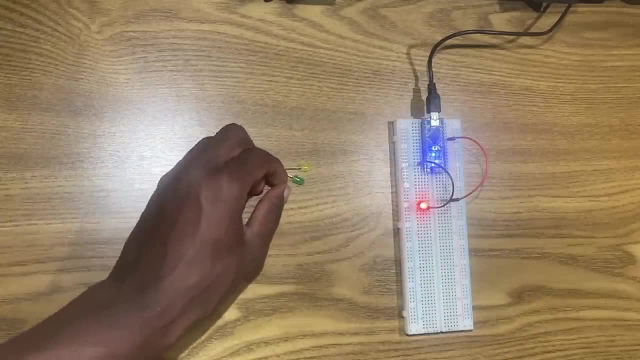 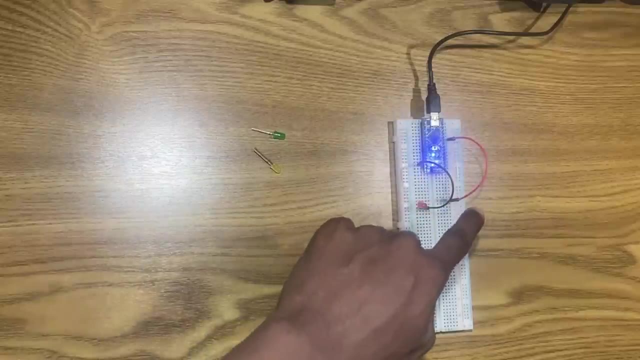 So what I wanted you guys to do is create a traffic light. So we have our green color right now, we've got our orange one and we've got our red one. okay, So we used one pin to set up. set up everything for one LED. 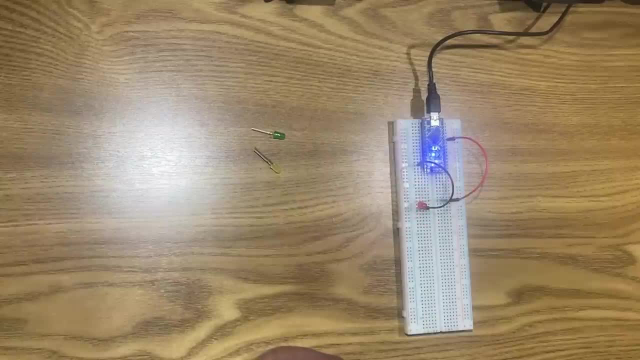 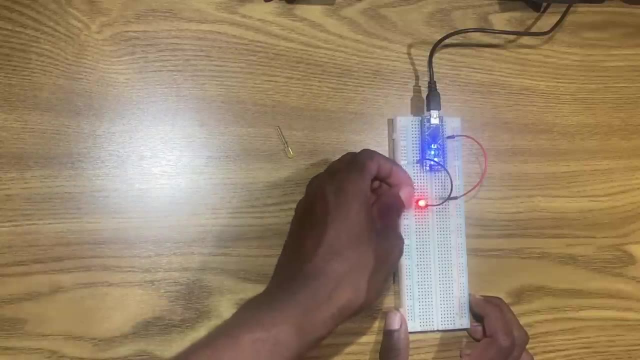 So how many pins are you gonna be using for three LEDs? You're gonna be using three pins, okay, So you're gonna be using three digital pins, So you're gonna put green in front. So, instead of actually the red one, green is gonna be right here. 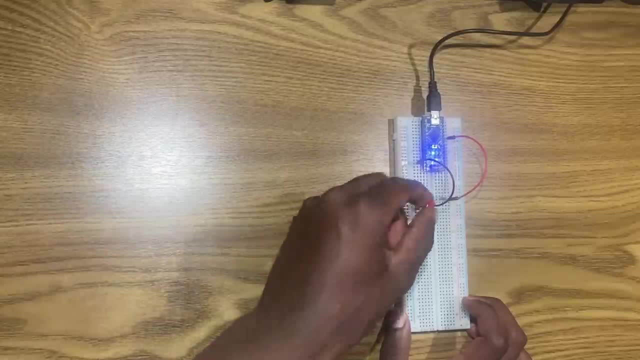 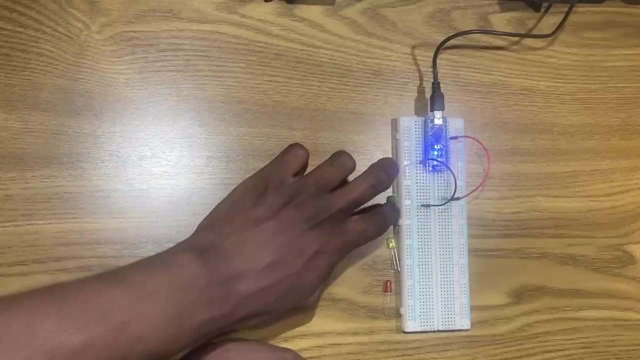 Then we're gonna have yellow and then we're gonna have red, okay, So we're basically creating a traffic light. So I want this to do is basically okay. What I want this to do is I want this to delay for five second and then turn off. 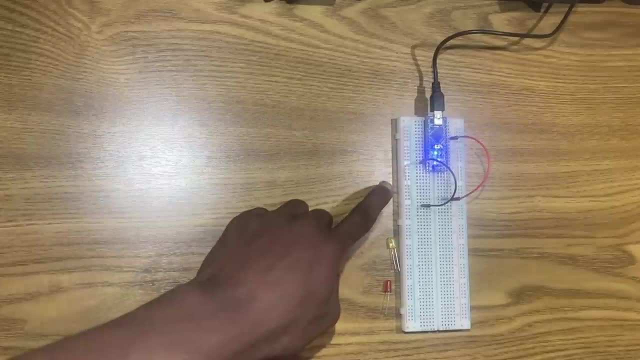 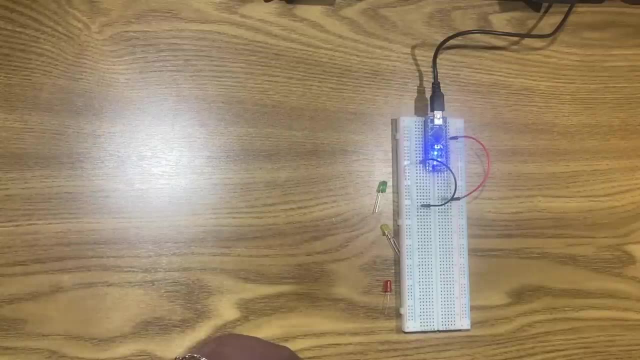 So it's gonna be on for five seconds, okay. Then when this one is off, obviously it's gonna turn yellow. For this case, yellow is a shorter one, so I'm gonna choose one second- And red- I wanna make it the same as the green light. 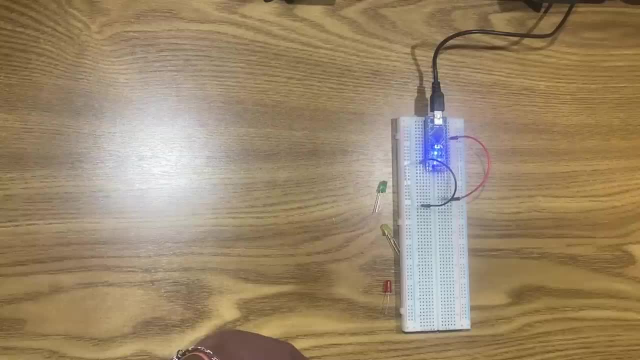 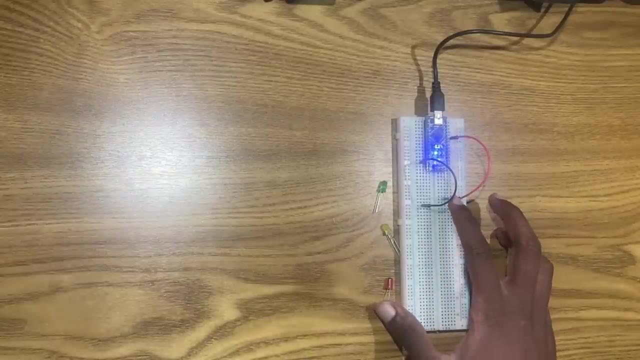 because that makes sense. So we're gonna make this five second too, okay. So I want you to create a traffic light, a working traffic light, okay, So you're gonna be using three pins, creating a resistor right here, using the resistor right here. 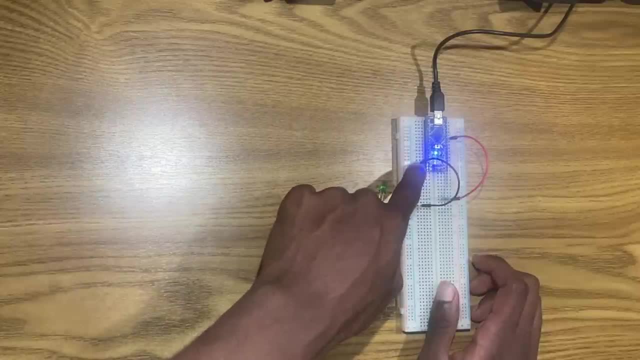 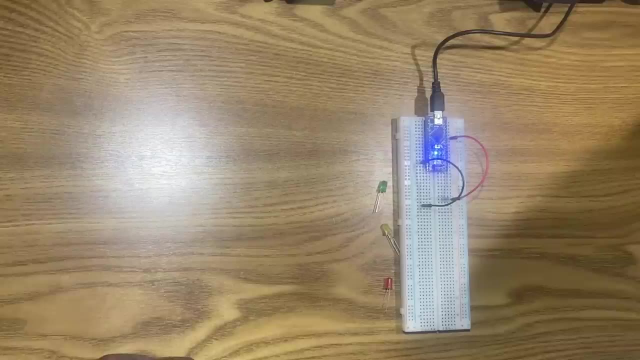 then obviously lighting up your LED, then going back to GND. okay, So they're gonna be using the same GND. So if I bring, let's say, a second wire, one thing you guys don't know is, let me just bring another wire. 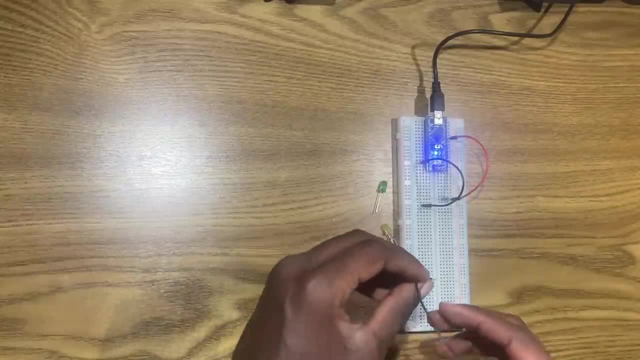 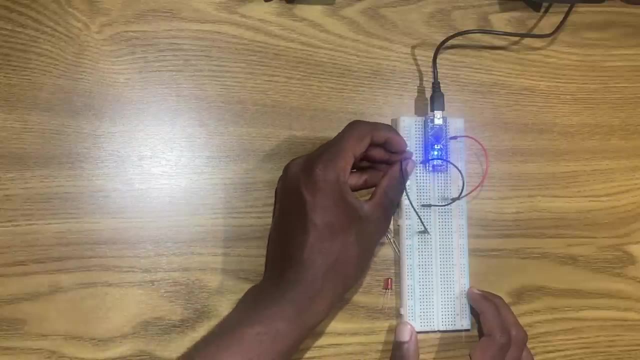 Okay, there we go, another wire. So let's say: I have my ground right here of the second LED, of the yellow one. let's say, for example: And what you're gonna do is connect to the same GND, okay, 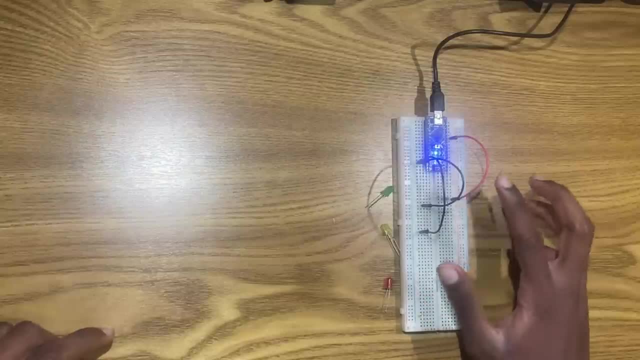 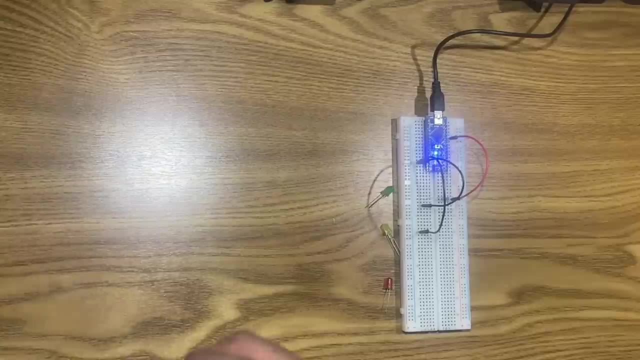 So you're gonna connect to the same GND. it's okay, But you're gonna be using what? Different pins? though? you're not gonna be using the same pin. You're gonna be using three totally different pins, So you might be using D5,, D7,, D8, it's up to you. 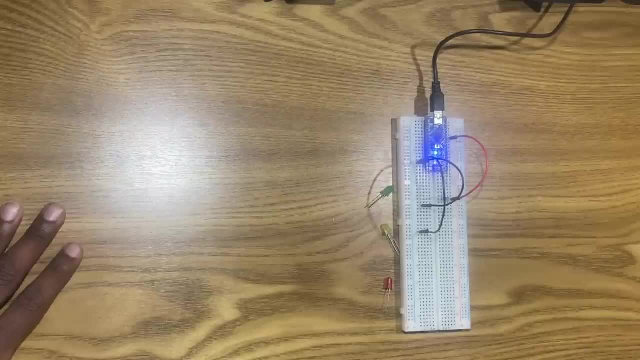 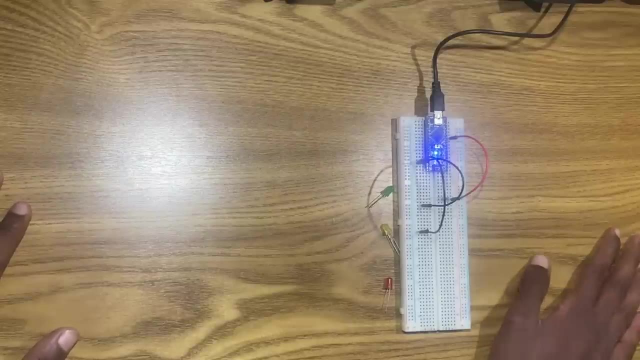 So, yeah, you're gonna be building this project for yourself. So before moving on to the next section, so pause this video and work on it. If you are not sure of how the circuit is supposed to behave again, you guys can use a digital simulator, okay? 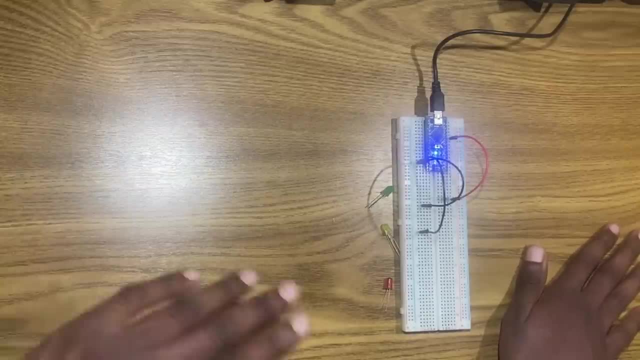 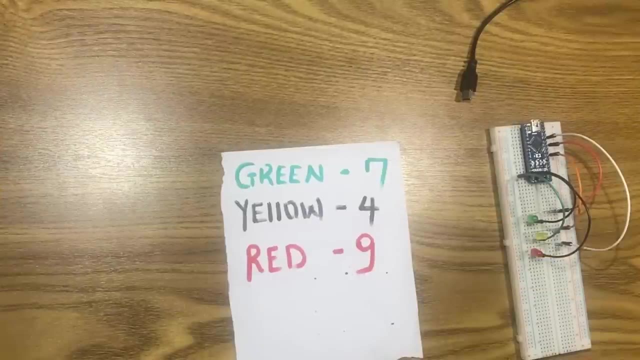 Afterwards. I'm actually gonna build it with you guys. In case you do not know, you can refer back to the next section where I'm actually gonna build it. Okay, so now we're actually gonna work on our homework, So I'm not gonna bore you guys out trying to build this. 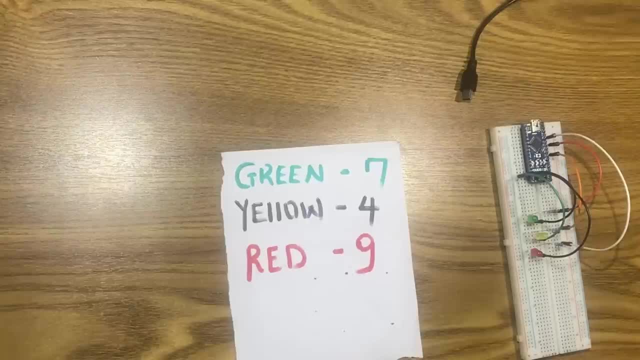 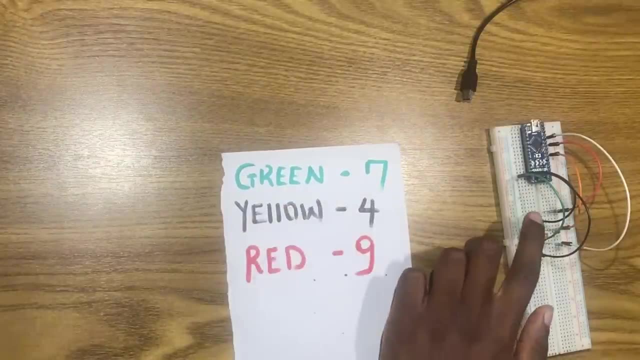 as I only need to use three different pins and do exactly the same thing. So the necessary information that you guys need is that green is connected to seven. So the green pin right here, the green LEDs- sorry, the green LED is connected to what? 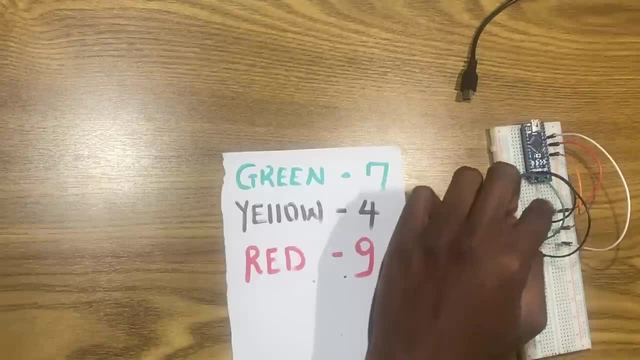 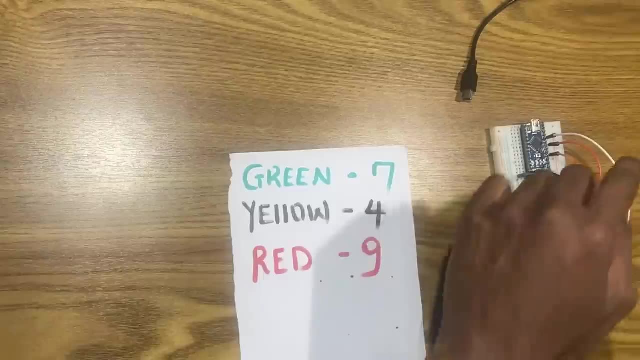 The pin, the digital pin seven. okay, So it's connected to what? The digital pin seven. The same goes for yellow. It's connected to the digital pin four, while the red LED is connected to digital pin nine. okay, That's the necessary information that you guys need. 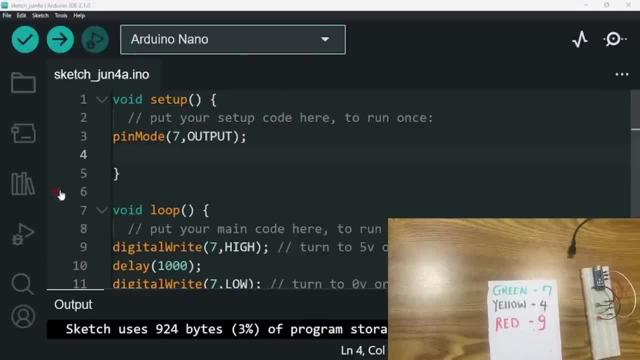 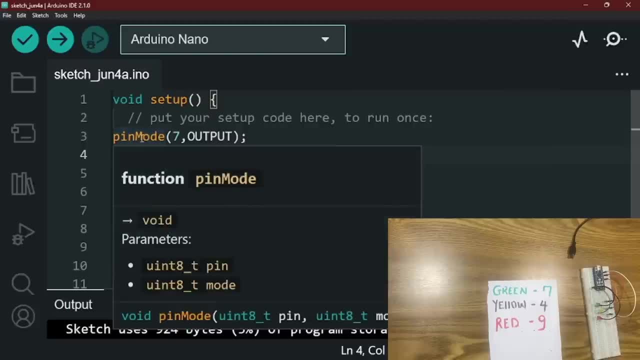 So now let's code this. So first we're gonna need to do a pin setup. So we're gonna need to go to pin mode and obviously set up our pins. So we wanna let Arduino know what pins we're using. So let me just copy this right here: 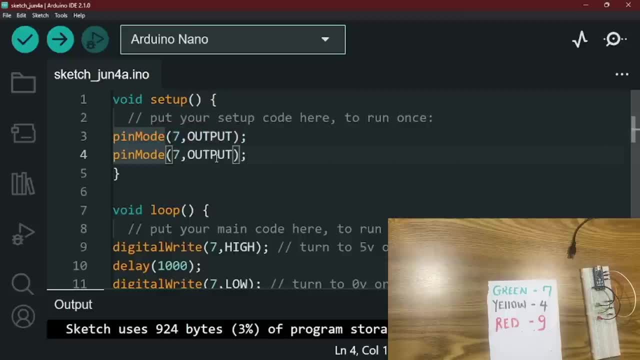 paste this and we're using pins, Pin four, so let me write down pin four right here. Four we're using as an output- Yes, we are. Let me again paste this- And we only have pin nine, So we're gonna use pin nine here too. 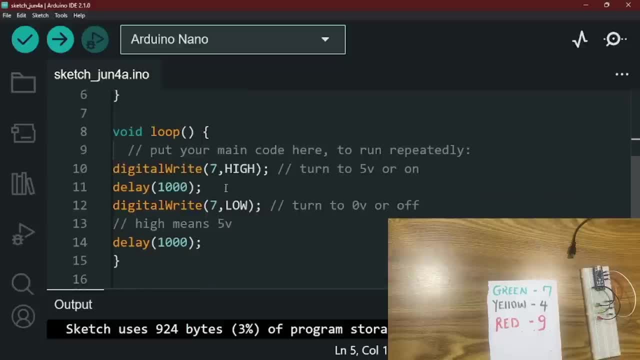 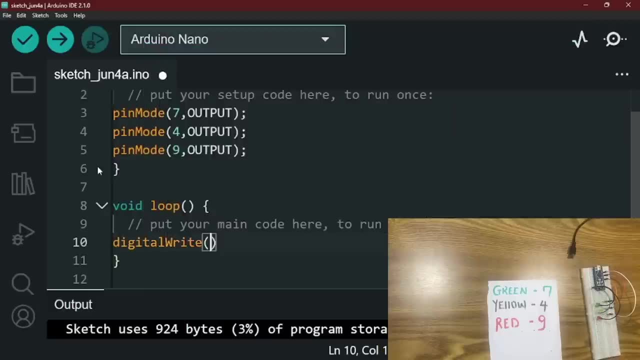 Nice, And once we're done with that, once we're done setting it up, let me just remove this code right now. So we're not gonna be using this, We're gonna digital light our pin. what Our pin? seven for green. 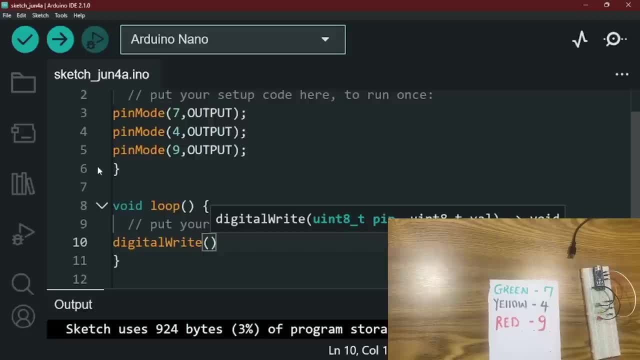 So we want green to light up first. So I'm gonna go for a pin seven, Then I wanna set it to high and finish it off with a semicolon, Then I'm gonna copy this again. Copy this, Then I want what. 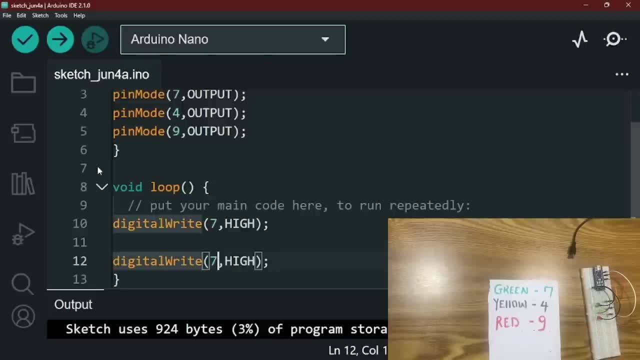 I want pin four to be high. But before that, actually before actually going to four, what do I wanna do? I wanna delay it. okay, I wanna delay it. for how many seconds? Five seconds, So it's gonna be 5,000 here. 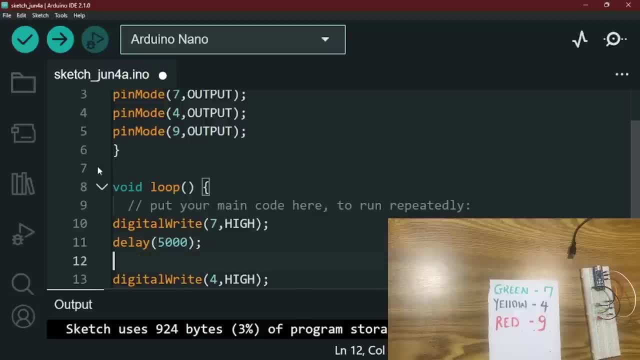 So I'm gonna be using milliseconds here: 5,000.. Then I wanna do what. I wanna turn it off, okay, So I want it to be low, So let me go here. They've got pin seven here. Then I wanna set it to what? 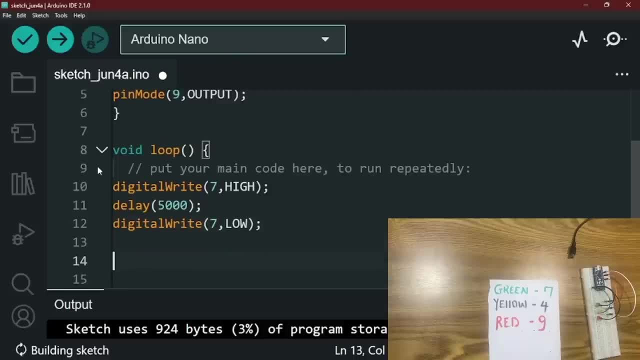 To low. okay, That's what I wanna do. Okay, when it comes towards the yellow LED, what do I wanna do? I wanna do is the same thing almost, but I wanna change the delay to what? To one second, don't I? 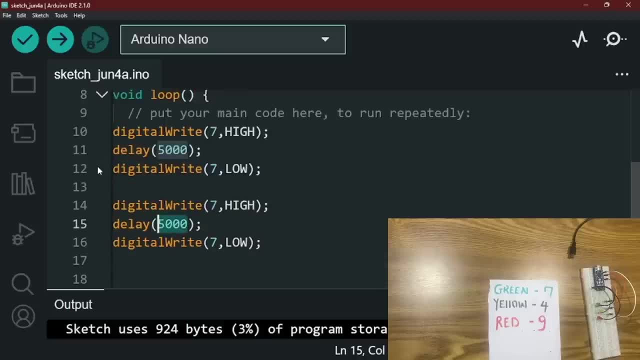 So let me see it right here. Let me set this delay to how many? One second or 1,000 milliseconds? And I wanna change the pin number again. I wanna change it to four. So go four, And I'm gonna go four again. 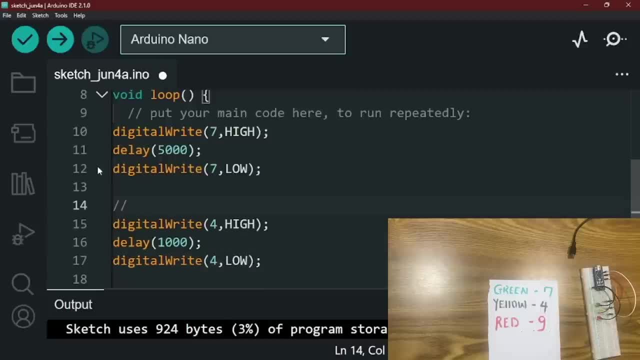 Okay, this is for what. Let me just write this description down, or comment: yellow. This one is for green, So let me write down green right here. Green. Then I wonder the red, what It's gonna be the same exact thing. 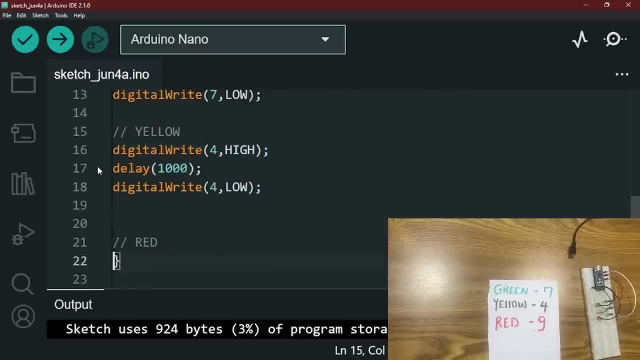 but I wanna change the pin with the green. Just copy that again, Do that. and I wanna change the pin number to what? To nine? okay, All right. So I think I'm done with this one, So let's check if it's actually gonna work. 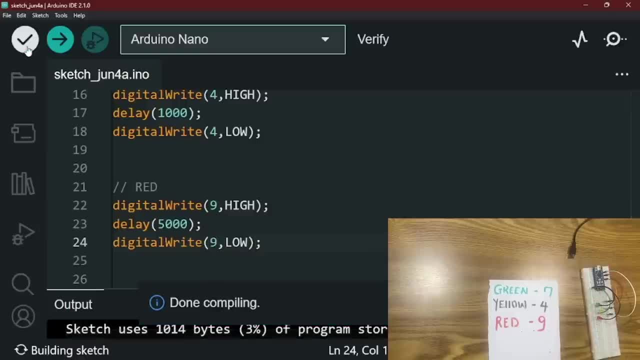 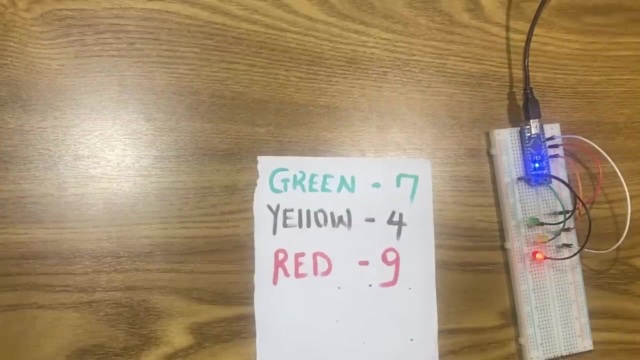 So let me verify this. Okay, seems like it's working. Let me connect my Arduino before uploading it. go here, connect my Arduino and let's upload the sketch. okay, it's done uploading, so let's check it out. there we go. there we go, it's working. nice, that's great and all. but if you look closely, let me go. 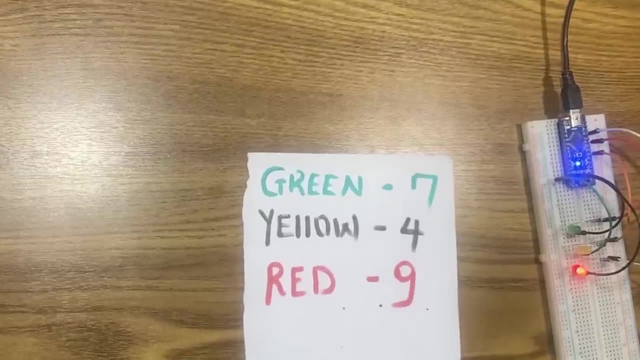 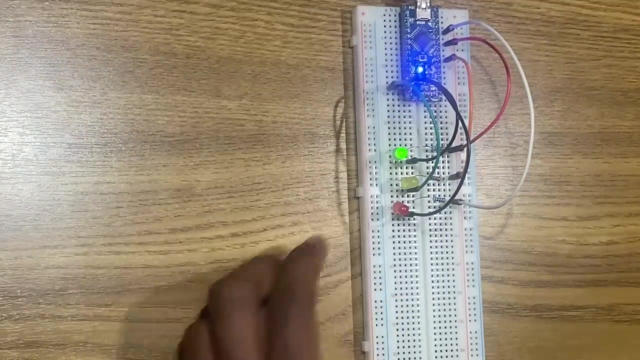 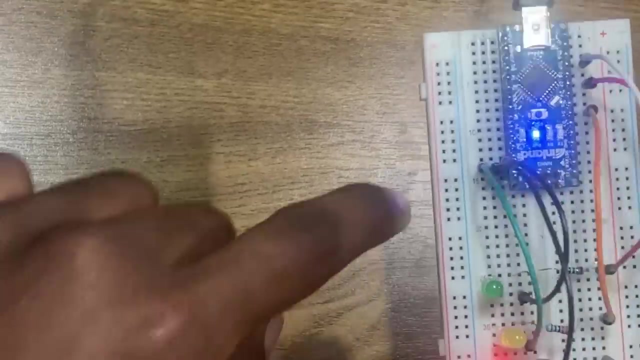 very close on my camera right now, like really really close. forget about this paper now, okay. so i want you to very look at this. let me bring it up close here, so if you look at it right now, can you see how much i stress the gnd- like it really looks really. 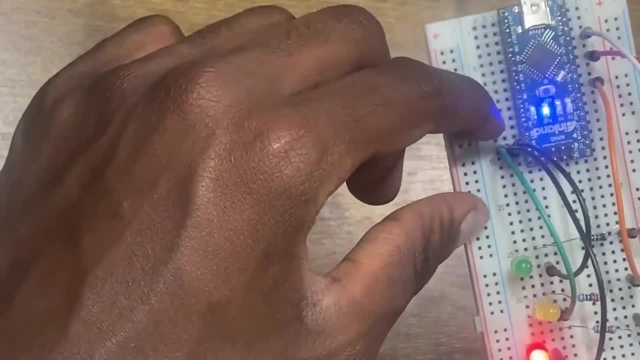 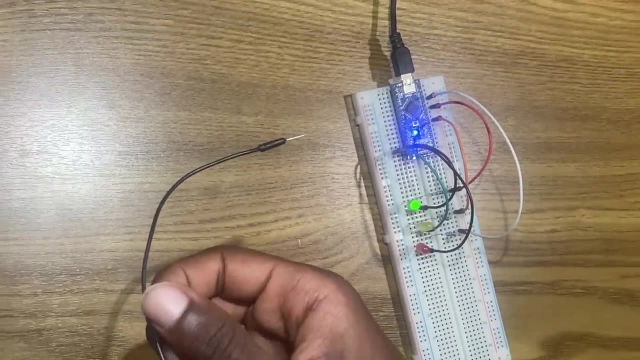 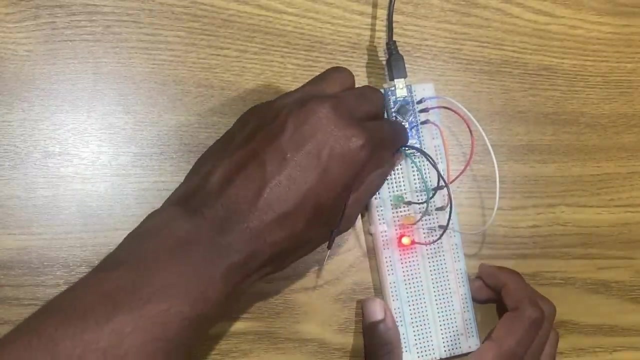 bad. this is, by the way, the gnd. all these three wires are connected to gnd. okay, so what can i do to fix this? so let me just bring an extra wire right here. okay, an extra wire, let me zoom out right now. for now, there we go. so i have this extra wire. what i'm gonna do is let me just remove this three gnd pins. 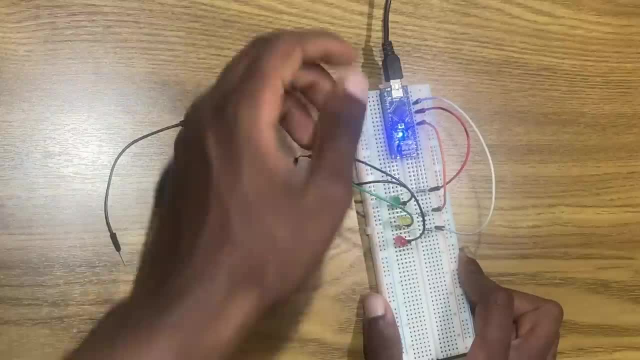 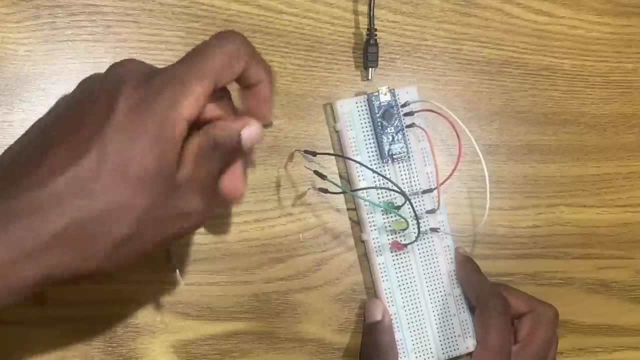 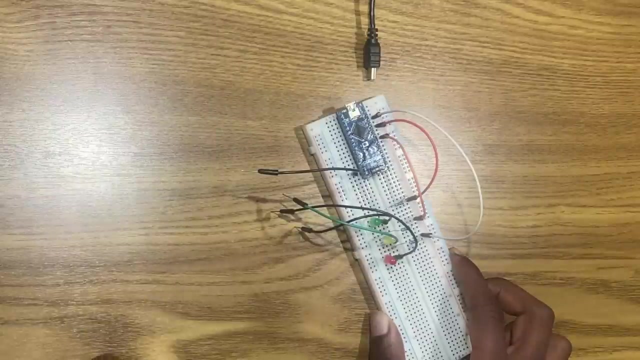 for now, before actually building the circuit. what do i want to do? i want to turn it off. i want to turn my Arduino off. first build and then we upload and then we run it. okay, so got my gnd pin right here. connect it. connect the gnd pin. if you cannot see it, i'm connected to the gnd pin, all right? 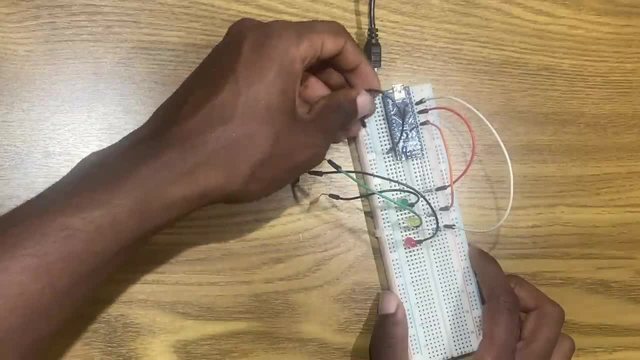 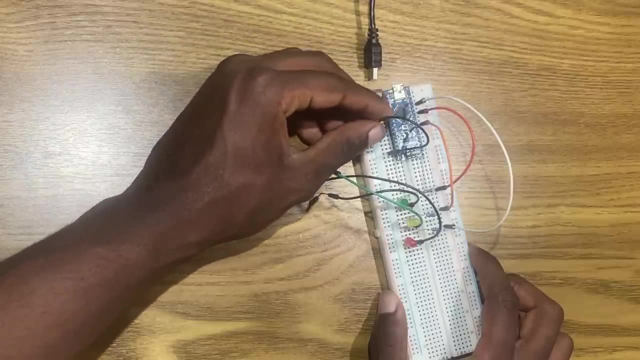 now, what do i want to do? okay, so i'm going to use this vertical stripe. can you see? it points to negative. there's a negative and positive right here. i'm just going to use the negative one as this. just again, convention, right, so i'm connected to this one. so, as i said again, when it comes to breadboards, the edge ones, 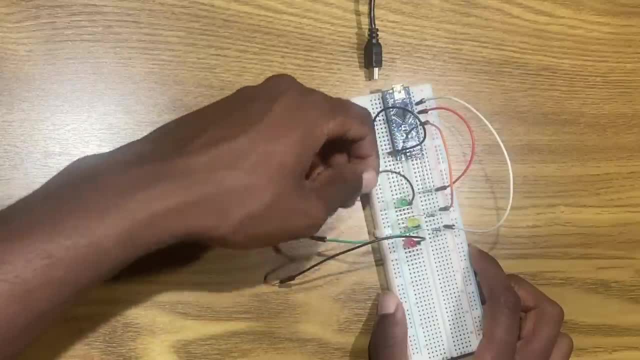 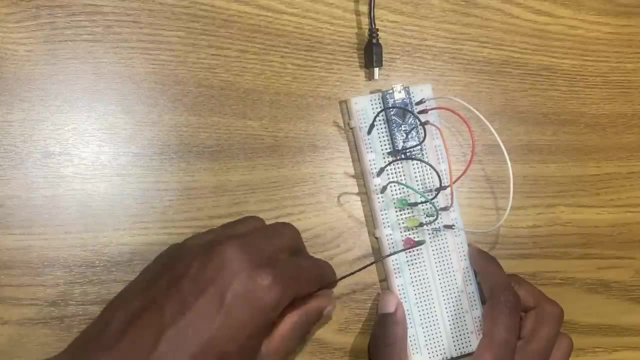 are connected all the way vertically, so i can basically do is what i can, just connect it to this one, the vertical line. again the same for this one. use this vertical line for the gnd pins and this one for the gnd pin. i'm going to use a vertical one. there we go. 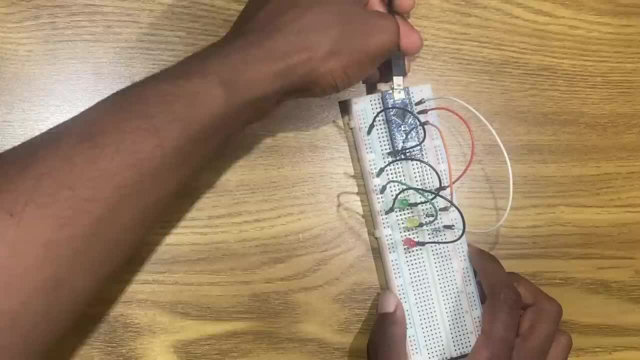 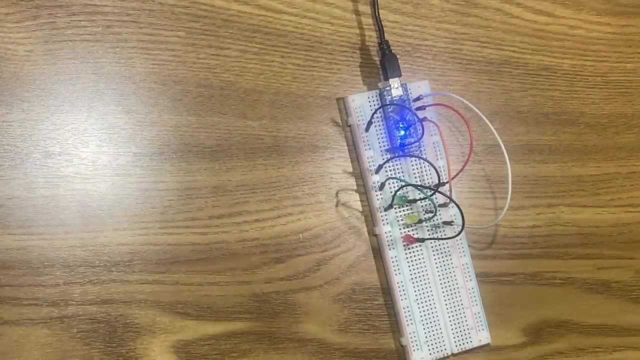 now it looks more nice. okay, so let me just again turn on my Arduino and run this. everything should be working normal. let's check it out first. okay, so five seconds, there we go. all right, it's working really really great. okay, so let's say i have a. 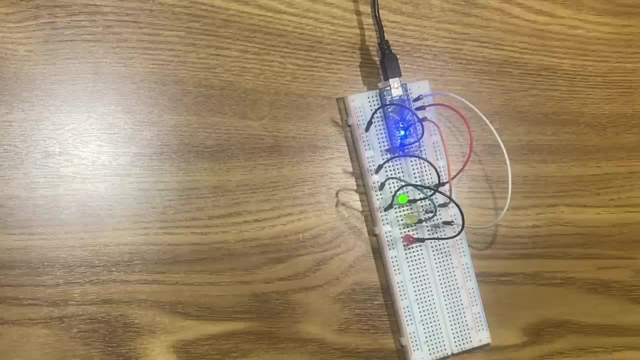 problem. i have to wait for like five seconds, and i just say it's just too long for me and i just want to use this in three seconds, okay. so what do? what should i do? i want to change the green and red to three seconds. i i like the yellow one. it's one second, it feels nice, but the red and yellow just. 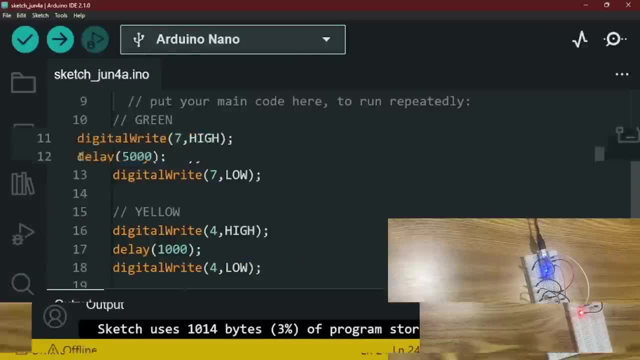 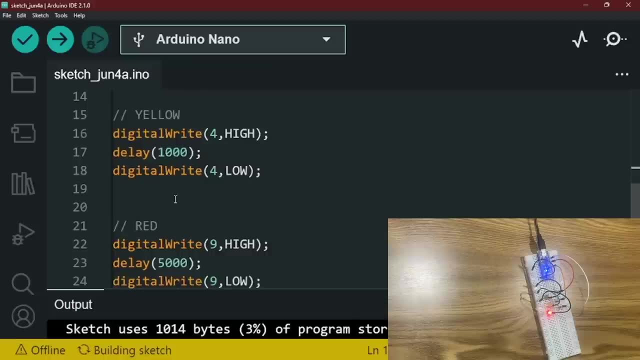 feels too long for me, okay. so what do i do? i go right here and change 5000 to 3000. not only that, too, i have to go back to red, then go change it to 3000 again. okay, then you have to upload it. 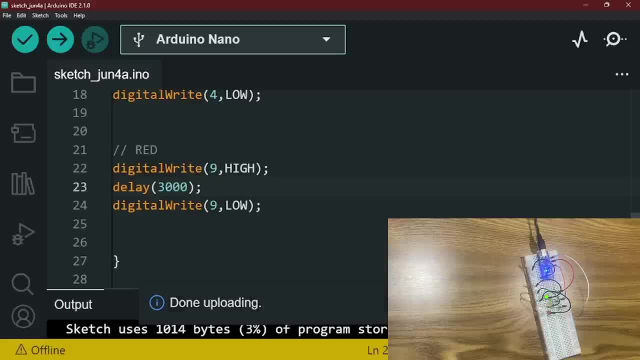 so it's going to work for three seconds now, but okay, let me just let's just check it out working. okay, there we go, it's working. okay, it's a bit faster. now let me just count again one, two, three and change over. okay, there we go, it's working pretty fine. all right, but i have to go change it in two separate places, so 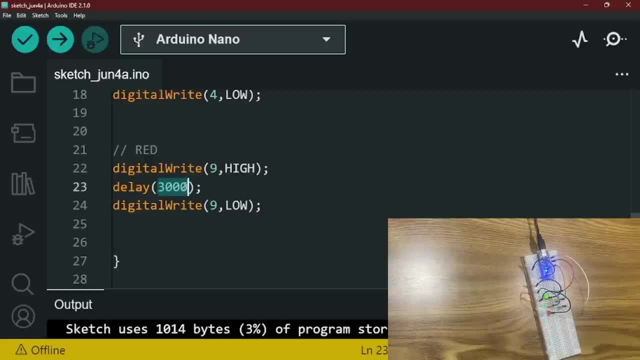 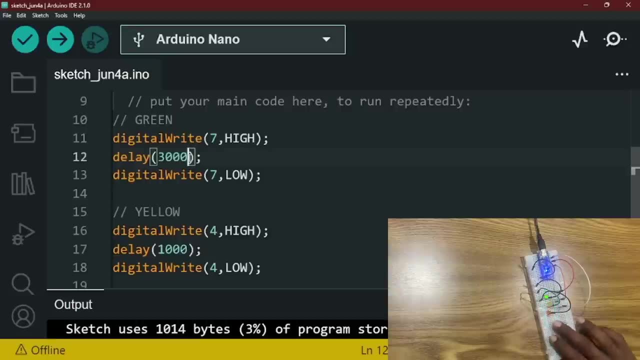 i have to go right here and change this to three thousand. again, three seconds. so i have to go right here again and change this to three thousand. just think of me having lots and lots and lots of leds right here. let's say i have five or six. i'm gonna have to go change it. what six places i don't want? 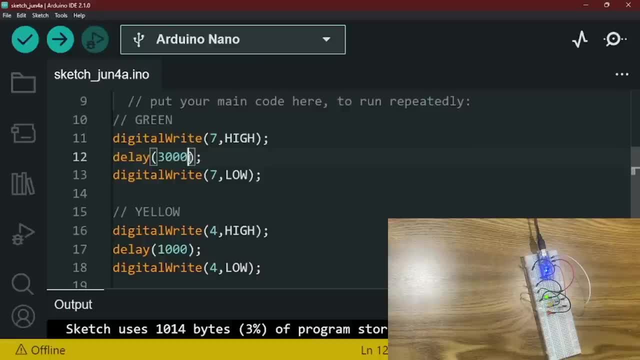 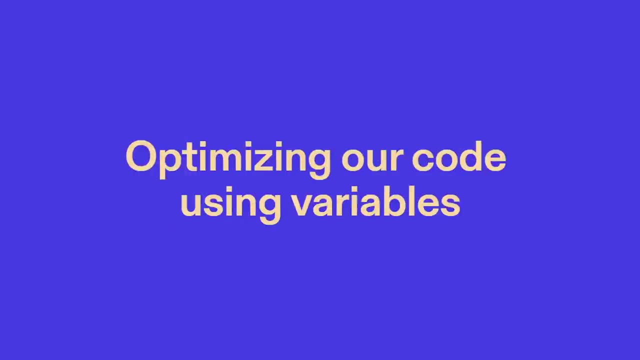 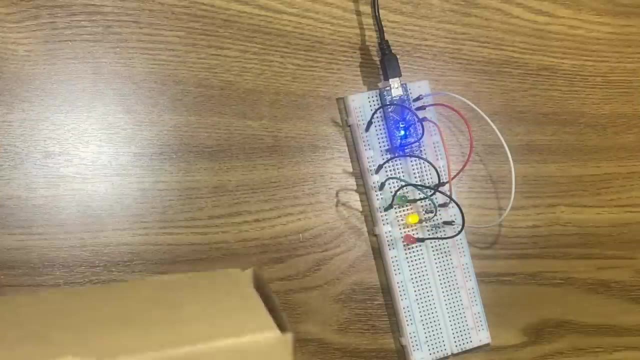 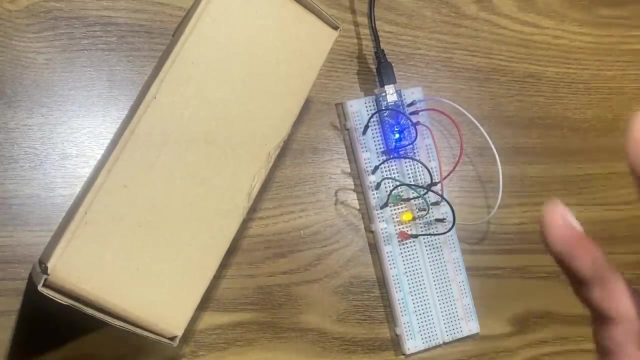 that to happen. so how do i do avoid this type of mistake? so we're going to learn something called variables. all right, so first, before learning about variables, let's talk about this box. so i have a box right here, okay, so this box, no label on it. you do not know what is inside a 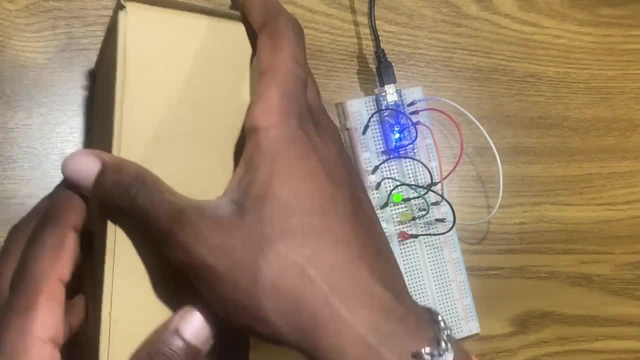 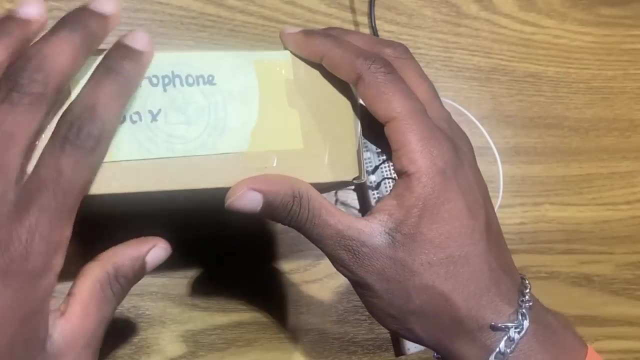 box until you open it. when you open it, you know what's inside. okay, so it has no label again, it's just empty. but to save us this effort, and let's say, i just checked it and labeled it right here and named it microphone box. okay, so i just gave it a label, so it's going to tell me what is inside. 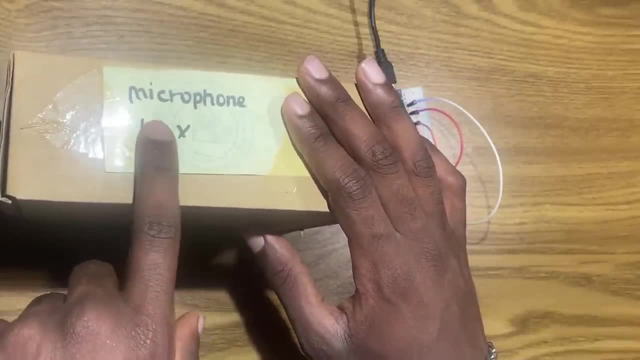 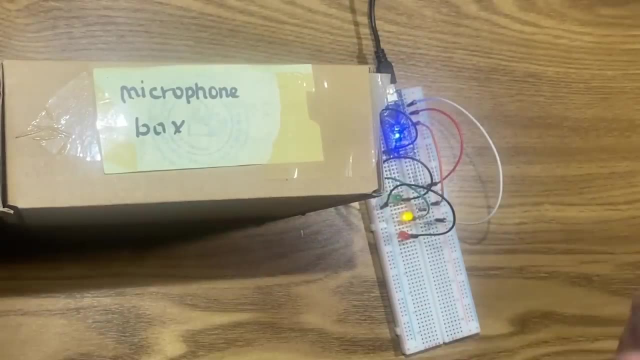 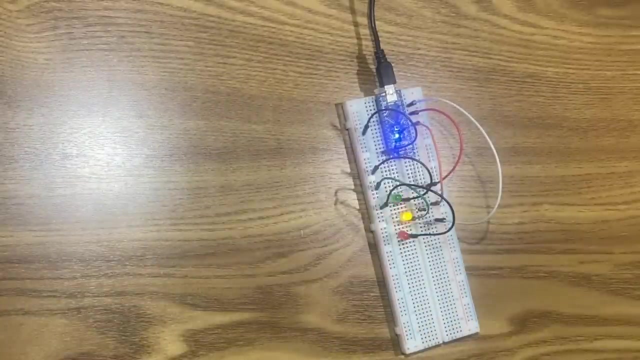 before even opening the box. so right now, by just reading this, i can say: is okay, this has some mic equipment inside of here, right. okay, this has mic before even what opening it, all right. so this is the nice thing about variables. so what they do is basically refer to things, all right. so they just basically: 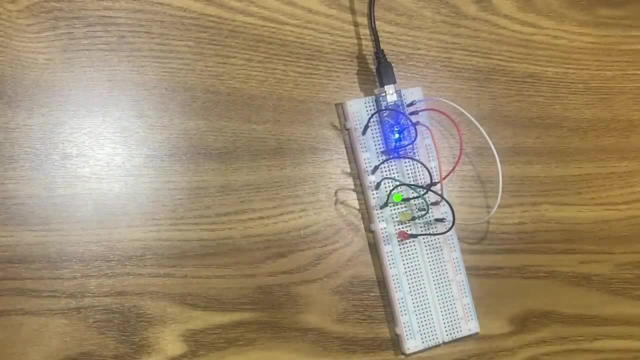 refer to our data, so we can refer to our data without actually changing anything about our data. our label does not change anything about our box. all right, it doesn't change anything. all it does is what? all it does is reference to our box. what is inside the box? that's just what it tells us. 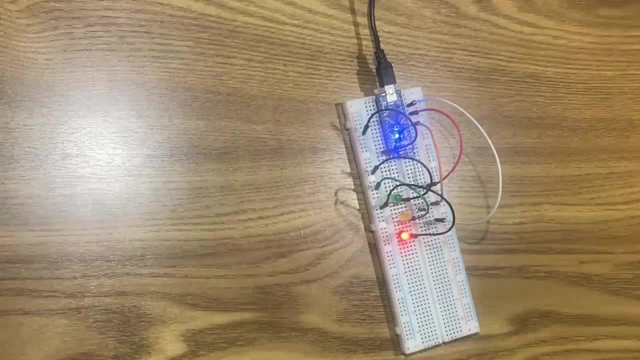 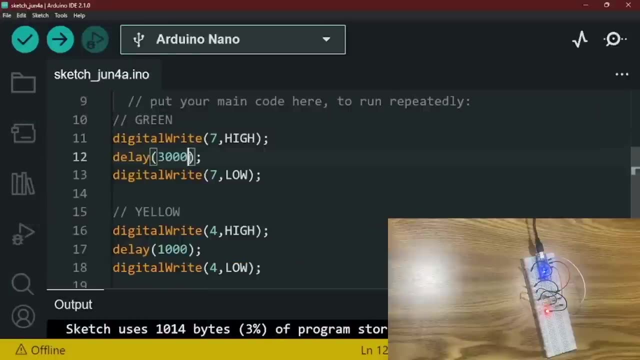 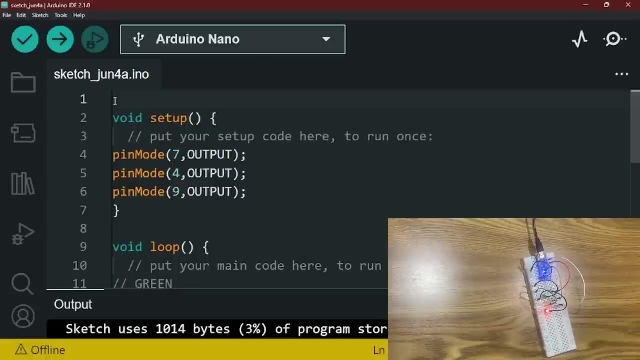 so how do we set up variables here? and we're actually going to see even a second purpose of variables. the first one is to reference things we're going to. we're going to check the second, the second, uh, use of variables. so let me go right here. let's see how you set up variables here. so all you need to do is go right here and use the. 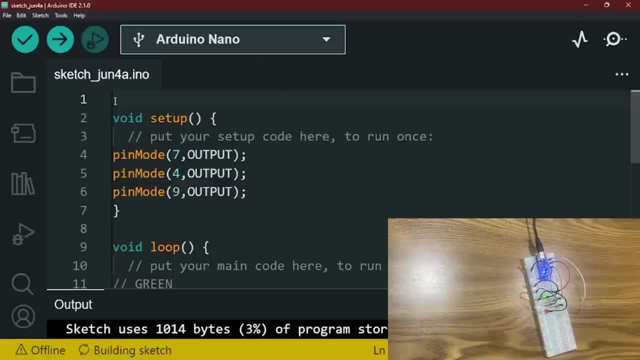 keyword let. if i correct, i don't think you use the keyword let here, so all you need to do is write down a name. so let's say, i want this to be delay time, so i just write down delay underscore time. okay, so i'm going to set this to 3000 and close this. 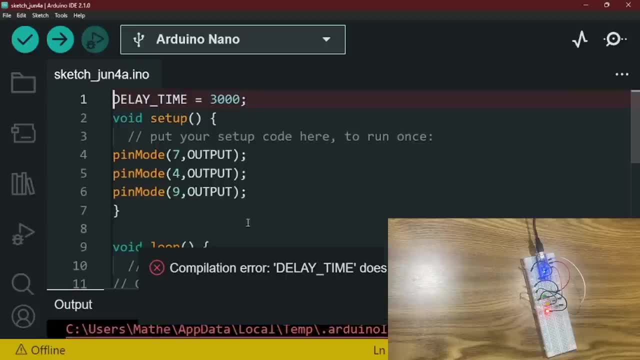 let me just verify if this is even correct and it says no, it's not, does not name a type. okay, so right here. all we need to do is go right here and say let let delete time. we do that. right here. let does not name a type. so you might be wondering. for those of you who are using 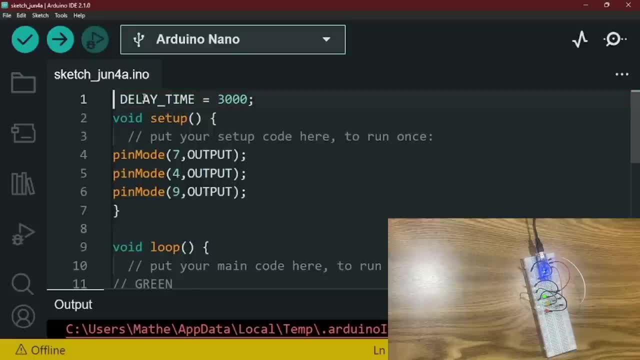 javascript and all that. we have to tell it what type of data we're putting inside. right here we're putting what We're putting- an integer, all right. So we have to let it know the type of data that we're storing, all right. 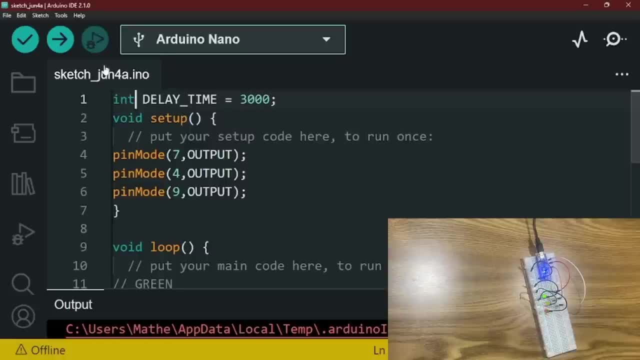 What we're going to say is int- integer. Basically it's an integer number. So let me just verify this again. It should be working pretty fine. now Can you guys see it? So we have to tell it the type. So when you're using Arduino, you're going to have to tell it the type of variable that we're using. 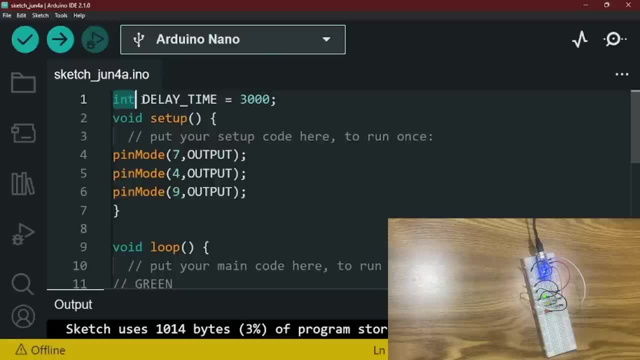 So in this case it's an integer I'm defining here And obviously I'm going to give it a name. So I'm going to call this delay time Again, this has nothing special on it, So I can just even call it something else that is unrelated to it. 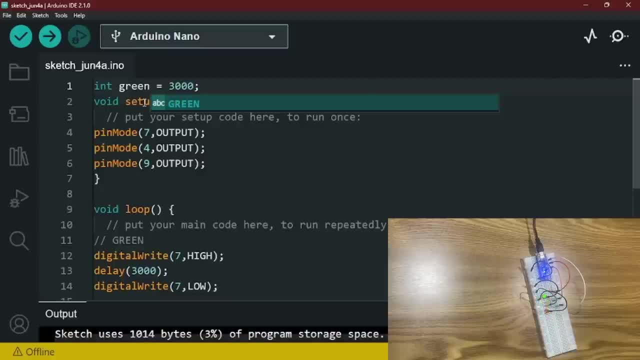 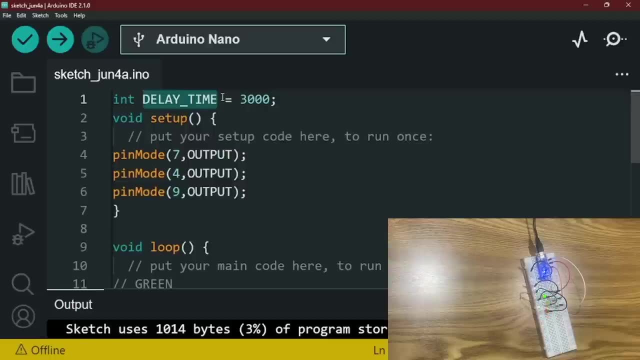 I can just say: you know what it's green. Or I can just say phone, Or I can just say anything, You get me. But I'm going to obviously put delay time, because that's what is the use of variables to give us a rightful information of what this is. 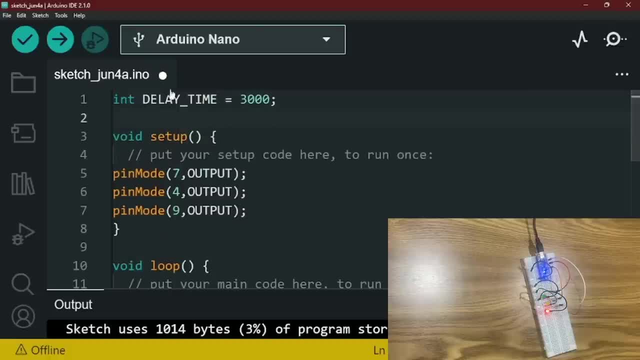 So even before somebody reading my code, they can understand before reading this code is that, oh, this is delay time, This is supposed to be the time And that is going to delay inside. obviously this again, this LEDs Okay. 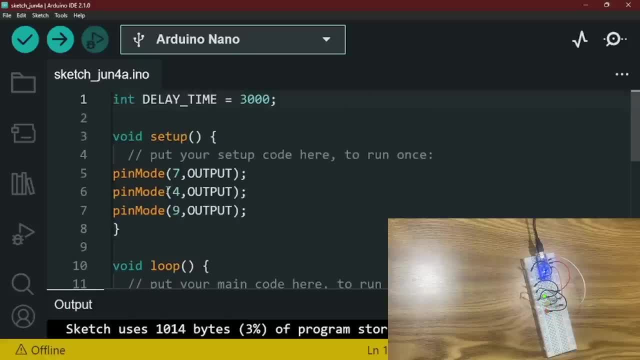 So I'm going to go say delay time and set it to 3,000.. All right, So let me just set it to 3,000.. So I'm going to remove this delay time right here, So I'm going to be using it. 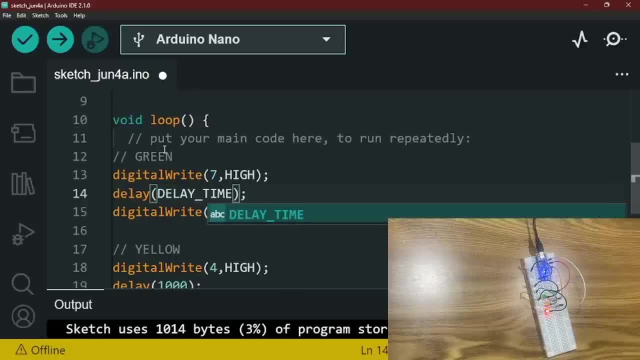 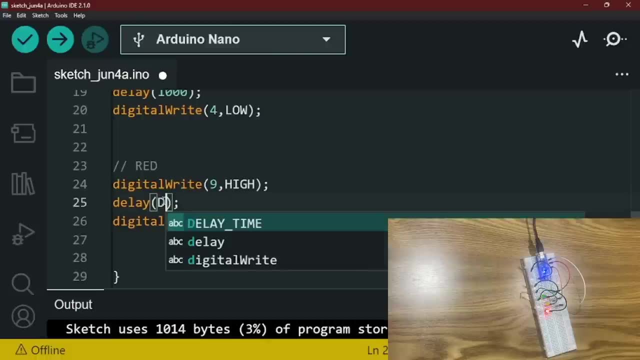 How do I use it? I just use it as a normal thing. I'm just going to say delay time. I already defined it. I can use it multiple times, All right. All right, Also for red. I'm going to go right here and use delay time. 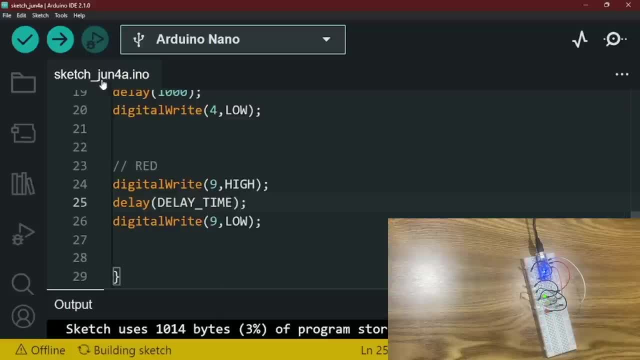 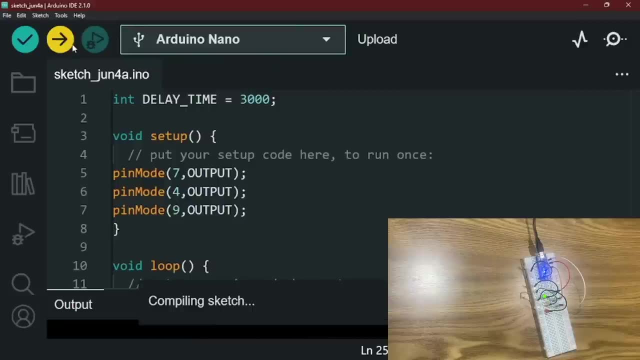 Underscore time. All right, Perfect, All right. That's all I need to do. If I verify this right now, I don't get any error. All right, Everything's sounding great. If I upload this, like I said again, a variable does not change a thing about what it's referencing. 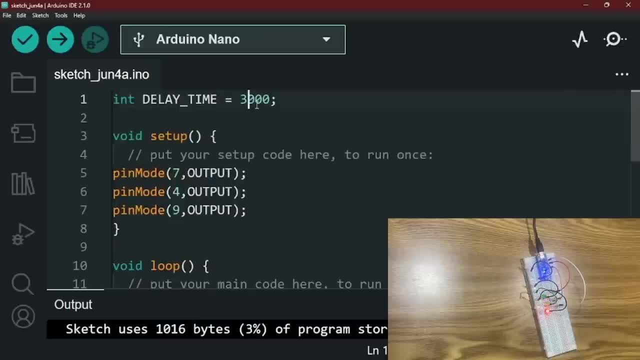 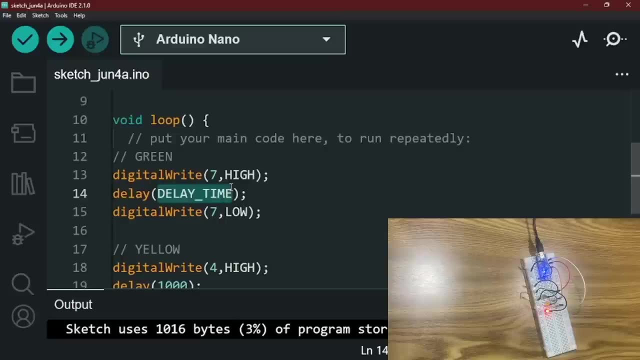 So I earlier said 3,000 here And basically what it's just doing is delay time is equal to 3,000 here, So it's basically putting 3,000.. The computer is manually putting 3,000 here, All right. 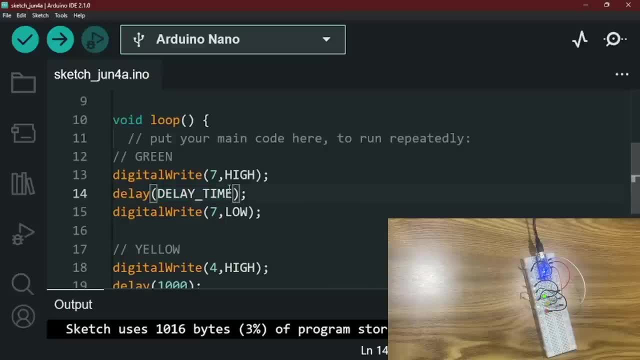 Instead of delay time. That's just what basically it does. So second usage of variables here is that. You know what? This is a bit too fast for me. This thing is just really fast. This is going three seconds And then one second. 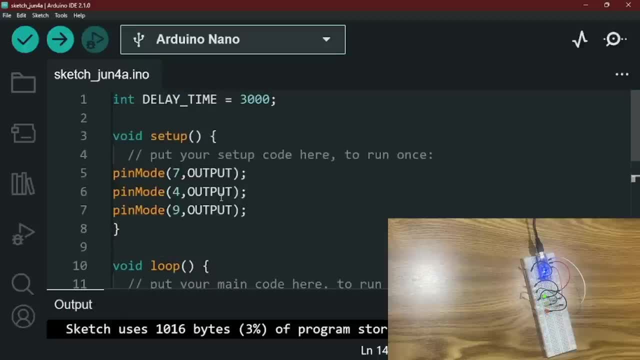 And then three seconds. This is very fast for me. I just want to make it four seconds, All right, So I can just do right here, Just change it from one spot. I don't have to go multiple spots to change it. 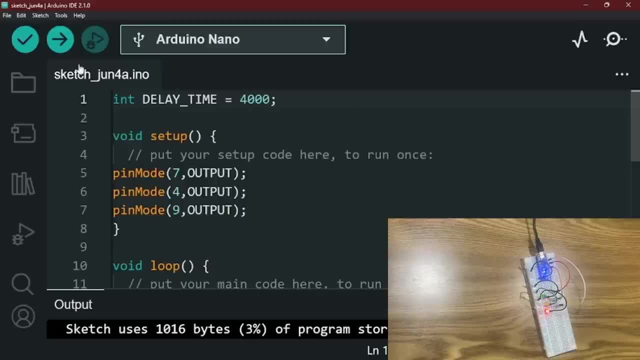 I have to find the ones. I can do is just change it from one spot and say: you know what? That's what I want. Let me just verify this. Let me upload this. I want it to be four seconds. I want it to be in the middle. 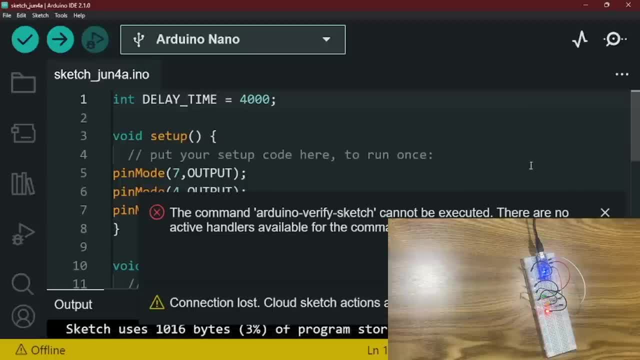 I don't want it to be too slow, I don't want it to be too fast. All right, So look at this. I upload this right now. It goes four seconds, So let me count this: One, two, three, four. 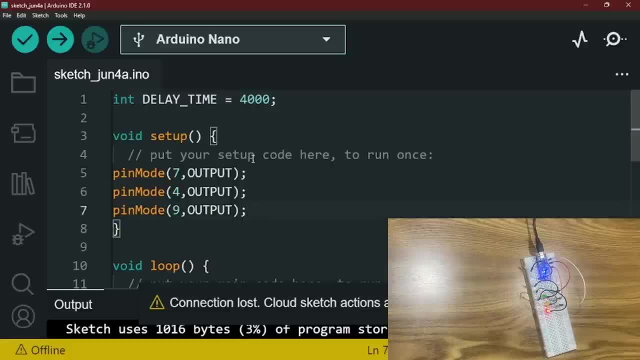 All right, There we go. So it goes for four seconds. All right, That's all you need to do. when it comes to variables, That's why we use them a lot, All right. So instead of using pin seven right here, just saying seven, four, nine. 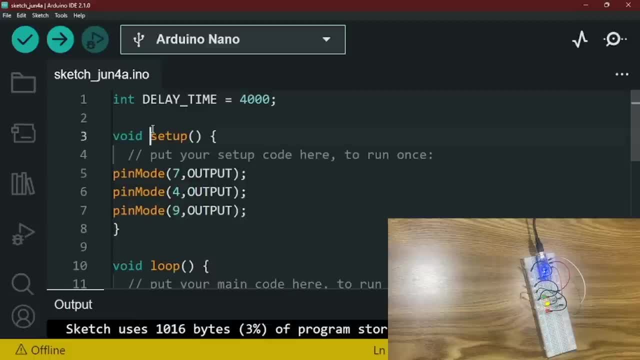 Okay, I can change it again for somebody who does not know what I'm writing down. before somebody even knows what I'm writing, I can write it down right here by just defining these variables. I just save them the time from reading the code. 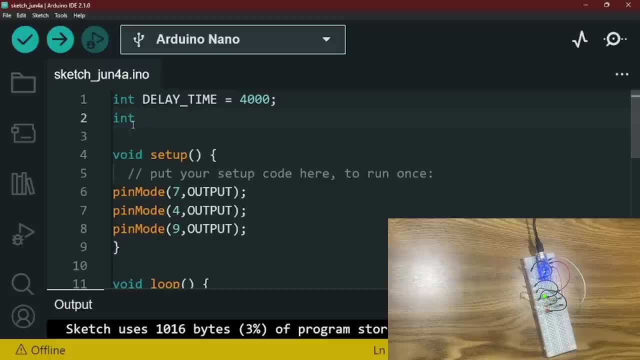 It can also work for yourself when you come back to this code. All right, So I can just say: is you know what I can call this digital pin? digital underscore pin equal to. let's see again, we have seven right here. 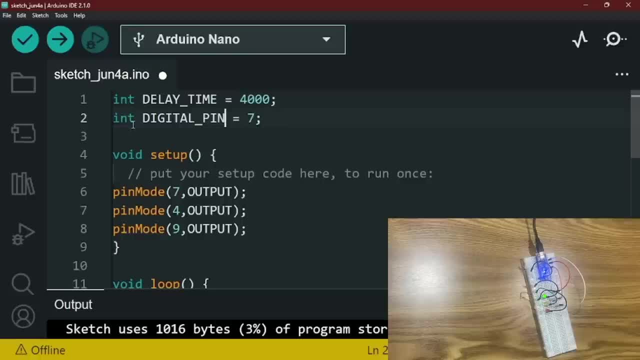 So there's still pin. let me just say seven, right here. All right, Let me see There's still pin seven, underscore seven. There we go, Then I again. I can write this down: Four, four. write this down for nine, nine here, four here. 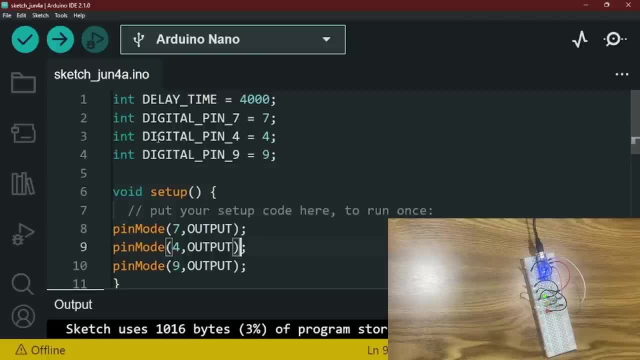 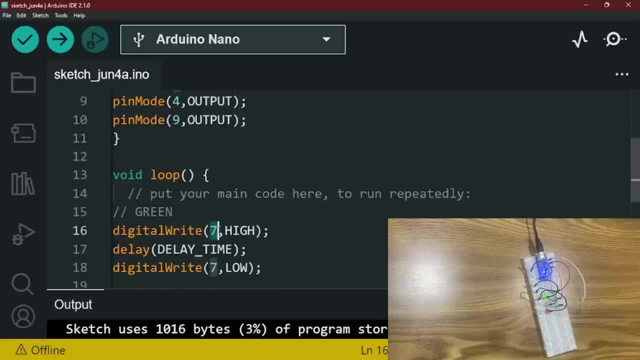 There we go And obviously replace this digital pins right here. So I'm just repeating pin, I'm repeating seven right here on pin mode and also on digital right. I'm repeating it over and over again. Can you guys see the difference right now? 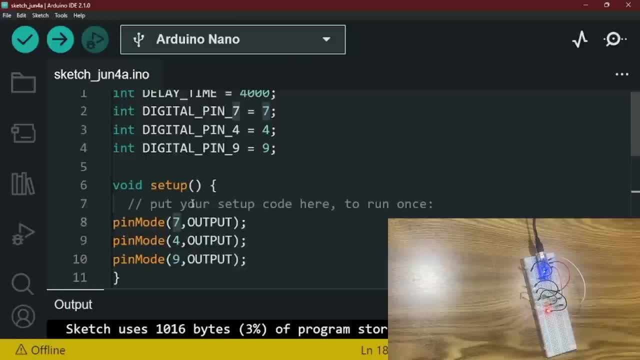 So let's say I'm changing a pin, I have to change it at three separate places. I don't want that to happen, So all I have to do right now is do the exactly same thing. I'm going to write down digital pin seven. it's going to have to complete it for me. 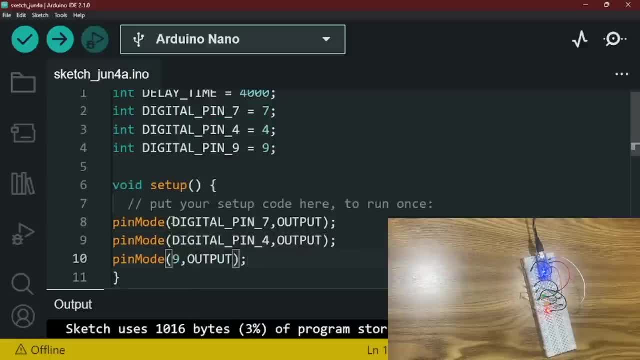 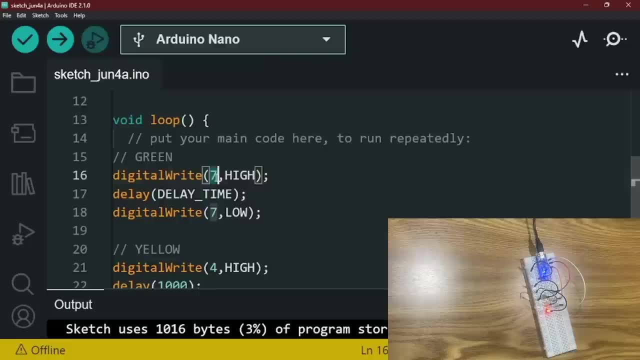 Then go say digital pin four and then digital pin what? Digital pin nine. Okay, So I'm just going to replace this again. So one thing you guys need to know is by using control D or command D, you can just select the same number over again. 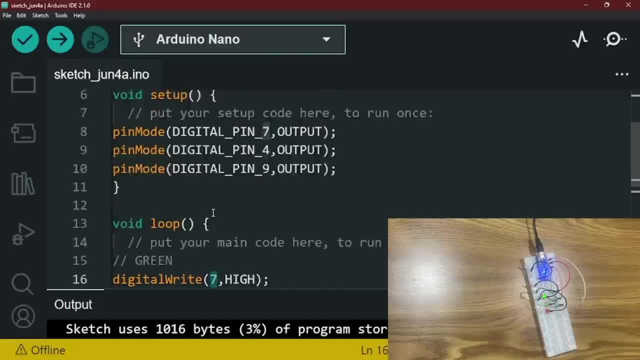 So you can select the same thing over again. Say, I'm going to select the seven right now. I even selected the seven from the digital pin, seven right here. So you need to be careful. So okay, I'm going to do is. 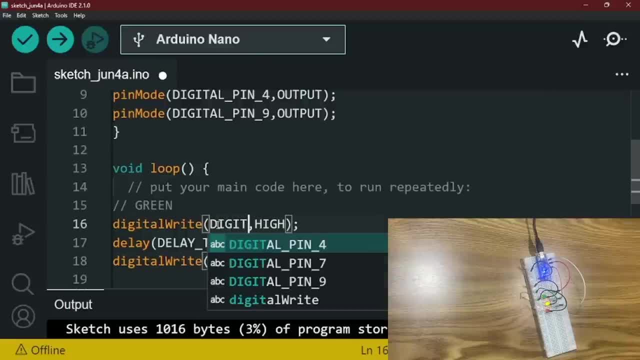 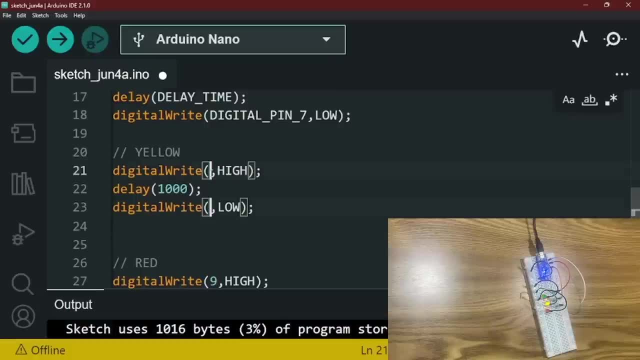 So, like this, two seven right here and I can edit them at the same time. Okay, Edit this at the same time. There we go. When it comes to four, I only have two fourths right now left. Do this. 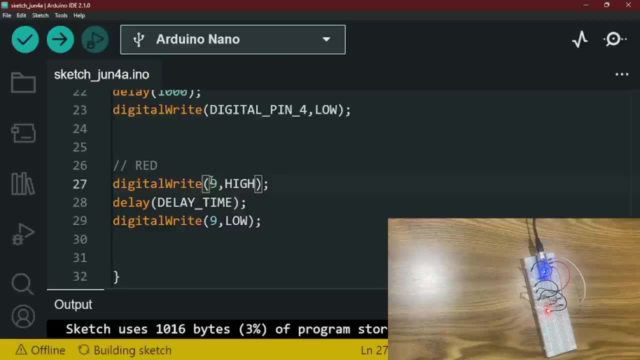 And again set this digital pin four, And when it comes to nine, I can use control D, select two, then digital pin nine. There we go. It's not supposed to change anything about our code, but it should make it. what a whole lot. 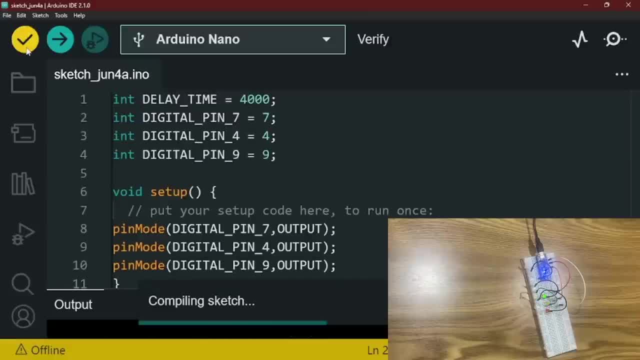 nicer and clean, All right. So let me verify this Again. if it's working properly, Okay, Everything seems fine, Let me upload it. Let's check if everything is working properly as it should. All right, Nice, Okay. 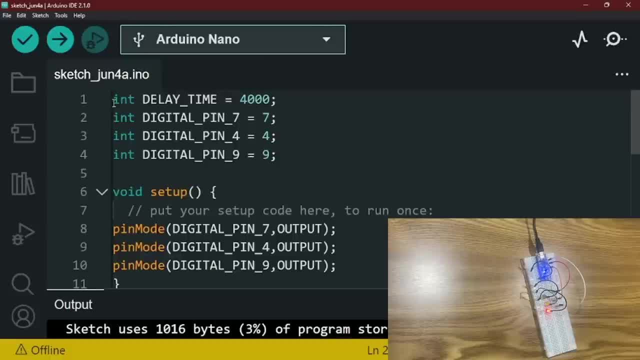 That's good, It's working really, really nice. So you guys learned about variables. So, again, as I said, one thing you should know about variables is, as I said, again, one thing you should know about variables is what they do not change anything. 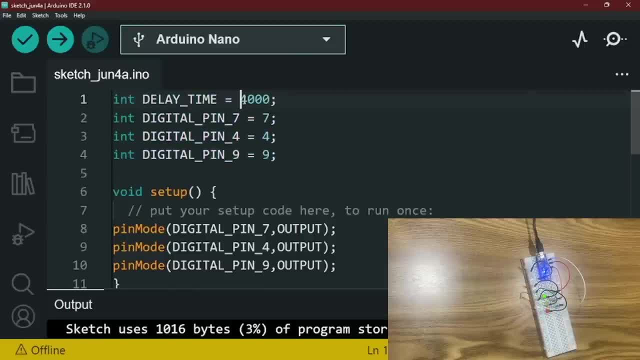 All they do is what reference? again, like I talked about the box, the label on the box, Just basically reference what is inside of the box, but nothing more than that. All right, So that's all with. comes to variables, So all they do is just refer data. 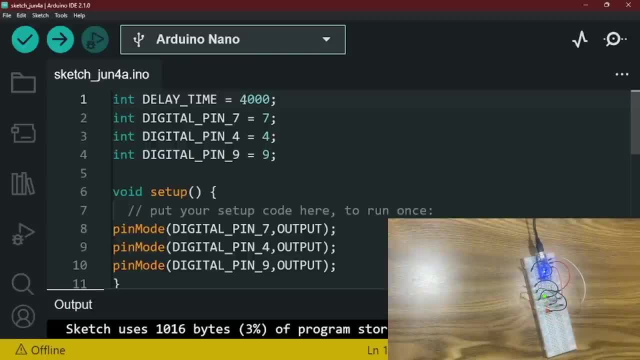 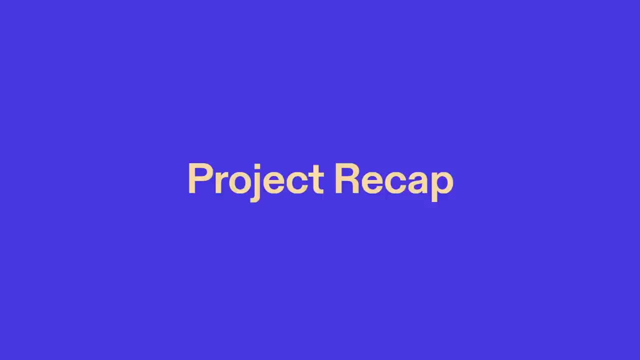 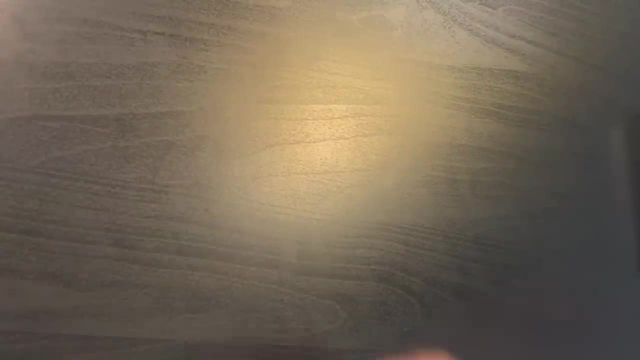 They just make it easier and cleaner to store data. All right, All right. With that in mind, let's move to the next section. All right, So let's recap what we've done so far. So at first, we began with the five volt, right here. 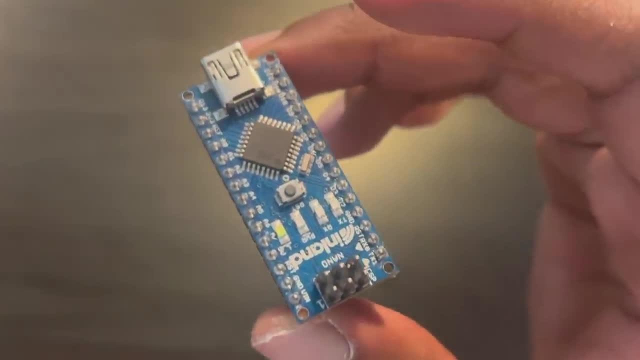 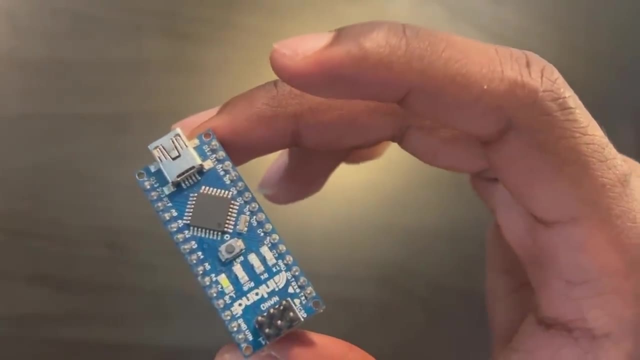 We began with the five volt and we built a simple LED circuit. Afterwards, we use these digital pins right here, And what we did is again build a traffic light. Okay, So what are these pins? marked with an A and a number next to them. 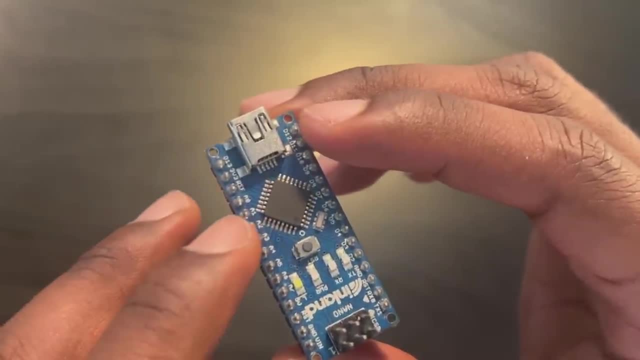 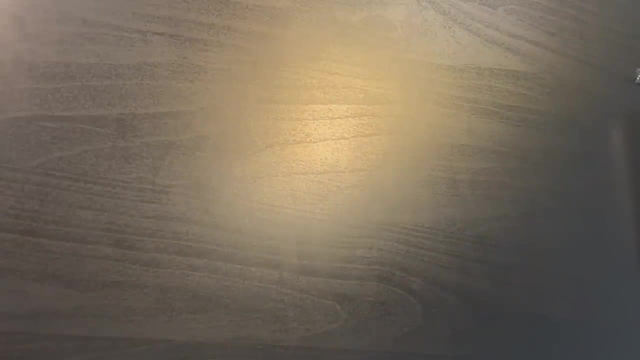 We're going to check them out in the next few sections. By the way, these are called analog pins. So in the next few sections, we're actually going to see the difference between analog pins and digital pins. Not only that, too, But we're going to see their purpose and why they are important in the Arduino world. 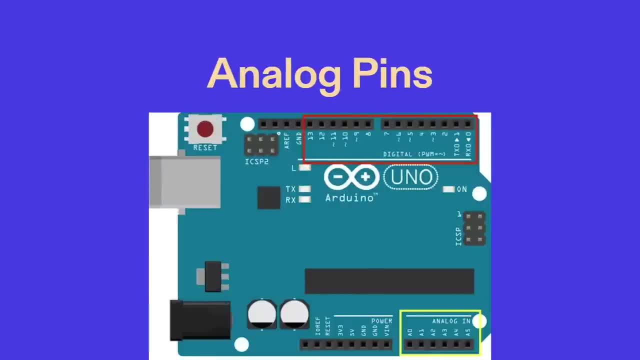 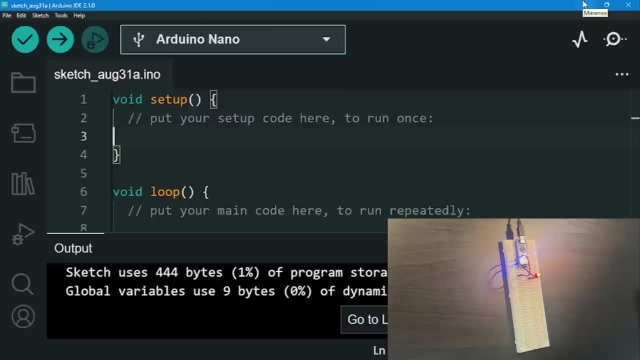 So see you then, All right. So let me show you guys what I did right here. So what I basically did right is that I set up the basic five volt LED circuit, So we have a five volt right here connected to the red connecting wire. 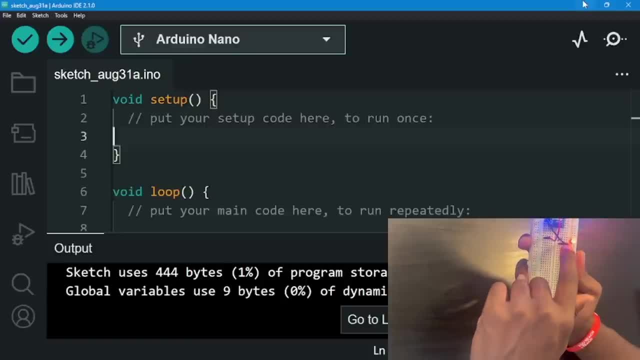 And then we have a resistor and we have our LED And then we go back to the GND with the black wire. That's all I did. That's what we did when we started this course, Okay, So so let me go over to my screen right now and let's start coding. 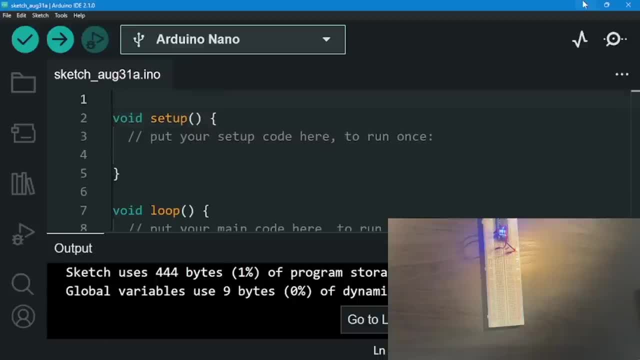 So right here, let me first give this a variable name. So let me see a red pin Right, Then let me give it a number. Let's say we're using pin four, right here, Analog pin four. Let's just say that again, I just took it by random. 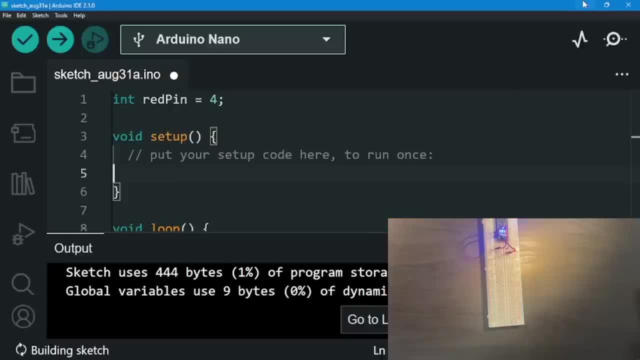 And right here, what we do is again as we did for digital pin. what we did was pin node. Then we put our what Our pin, which pin it is, And then how do you want to use it? Do you want to use it as an output or as an input? 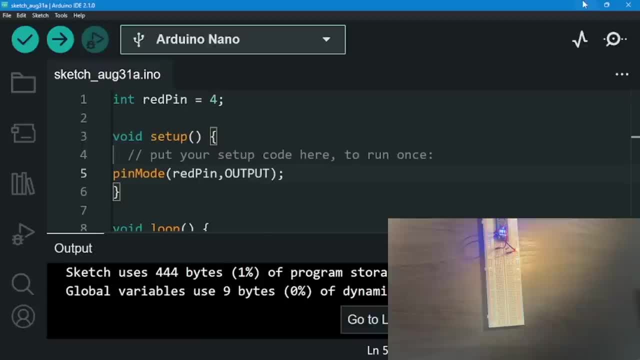 Always put a semicolon at the end of each line. All right, That's what I did, right here. But there is a problem right here. So right here, When we're using digital pins. right here we did was only put the number. 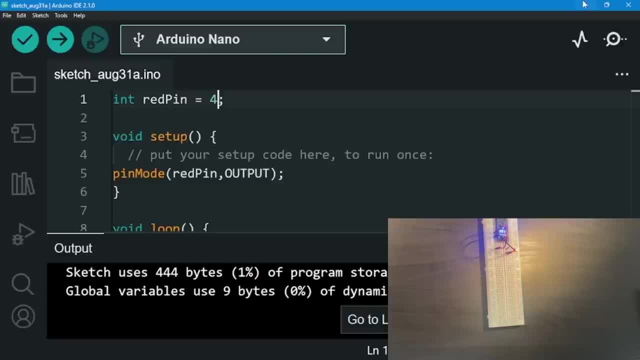 Right. So let's say I'm using digital pin four, right here. Let's just say that I'm using digital pin four. I'm doing that. What happens when I'm using digital pin four? What I did was just put a number right here and set it up like I did for an analog bit. 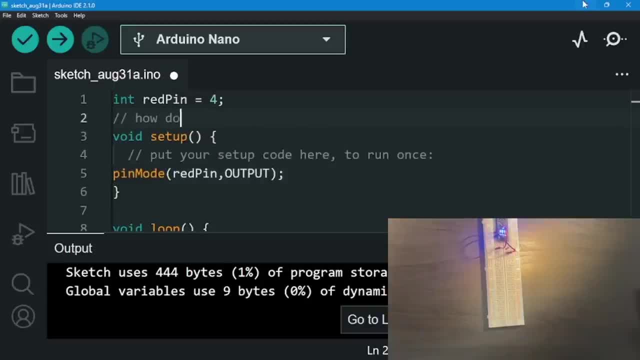 So, right here, how do we know the difference? We know the difference between digital and analog pin. so how does Arduino know that we're using digital pin four or analog pin four, right here, Arduino does not know. OK, so every time to differentiate an analog pin from a digital pin, what we do is put capital A for it. 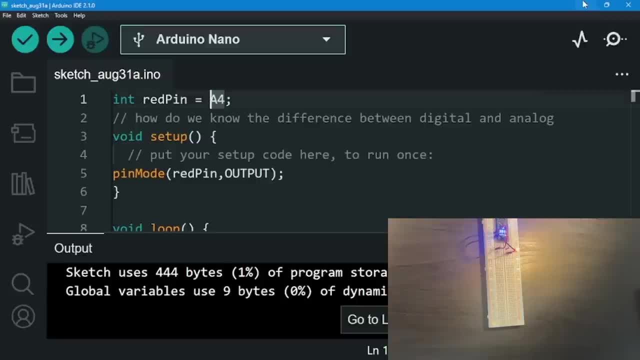 All right, Before the number that we're going to use. we always put a capital A, All right. So it's going to differentiate and we're going to know actually which pin we're going to be using. So, right here, Arduino will not be what will not be confused if you want to use the digital pin or the analog pin. 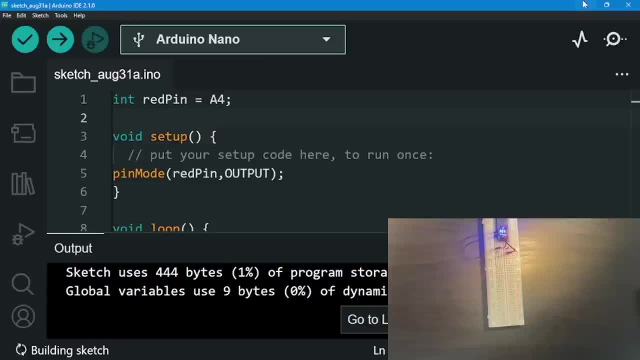 OK. so we're going to do is what? Put a capital A beforehand, All right. So once I'm done setting up the pin mill right here, what I need to do is go here, All right. So what did we do, right here? 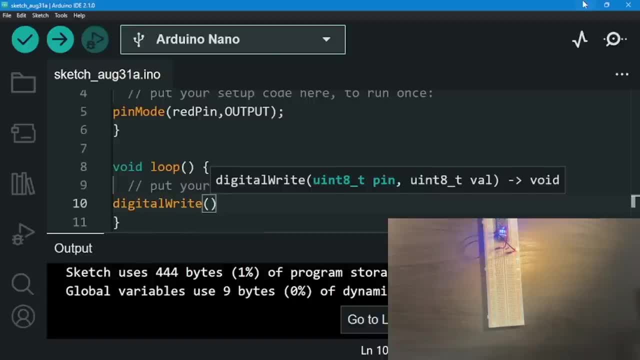 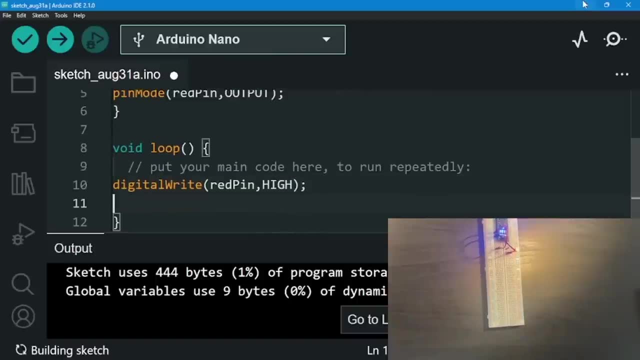 We said digital, right, and we set it to what. What do we do? We put the red pin right here And then we set it to high when we were using additional pin. So right here it makes sense to write what analog pin is, something called analog. 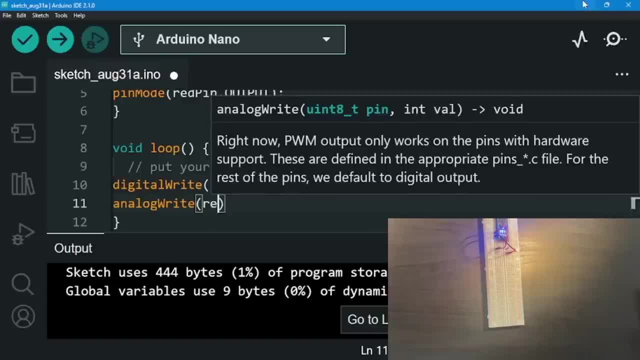 OK, we do that and we see a red pin- OK, the pin that we're going to be using- and then we're going to put a value. So, right here, I'm just going to put 255 and I'm going to come back to this and actually explain why did we put 255. 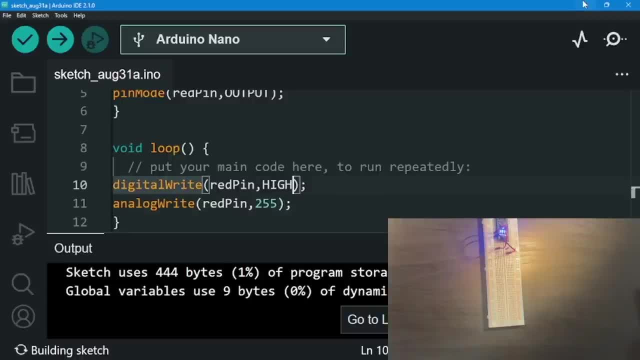 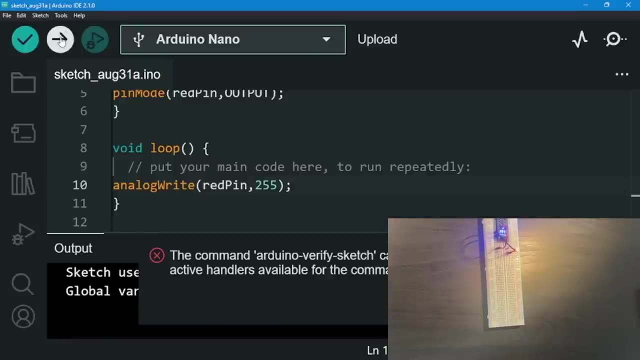 So let me just remove this right here, because obviously we're not using it, Using a digital pin. right here, let me remove this And all right. So let's verify it and let's upload it. OK, Right here, And it's done compiling, it's uploading and it's done uploading. 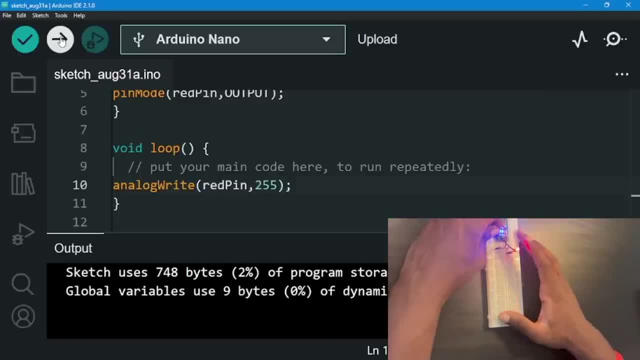 All right. So let me remove my Arduino from the five volt and let me move it towards the digital pin. not digital pin, Sorry, I said analog pin four. Let's do that. And there we go. I moved it to analog pin four, right here. 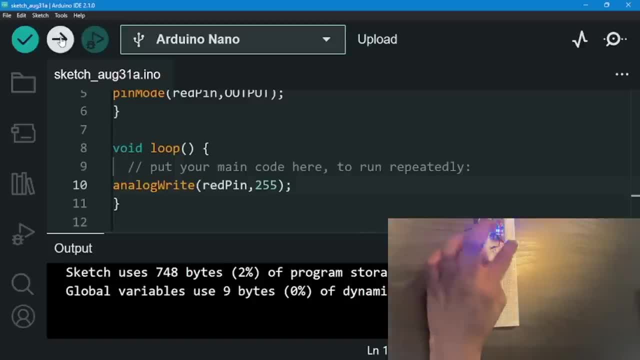 All right. So right now it's lighting up as how a five volt lights it up, and it is still a digital pin lights up the LED. So again, you might be confused on why did we use 255 right here? What is the use of it? 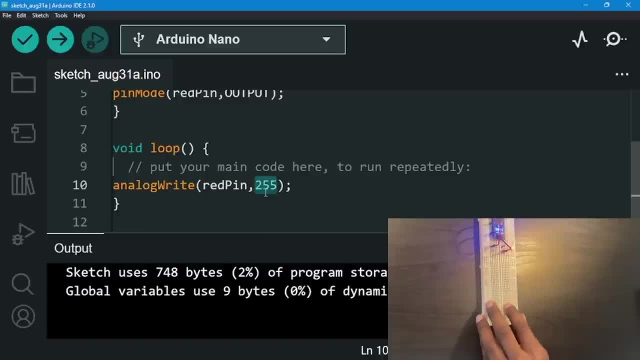 Not only that, too, but what's? it's a very odd number, you know. why not 300?? Why not? Why not? Why not 200?? Why 255 specifically? OK, so let's see the science behind it to understand why it is 255, and 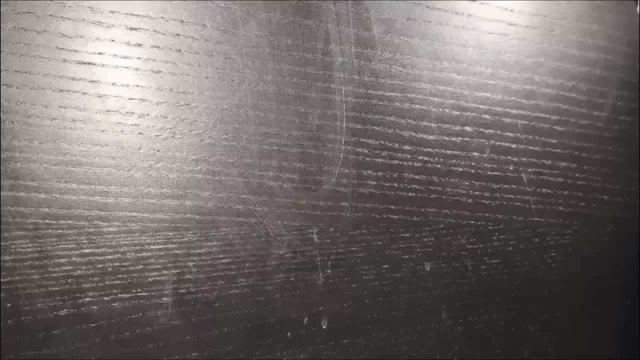 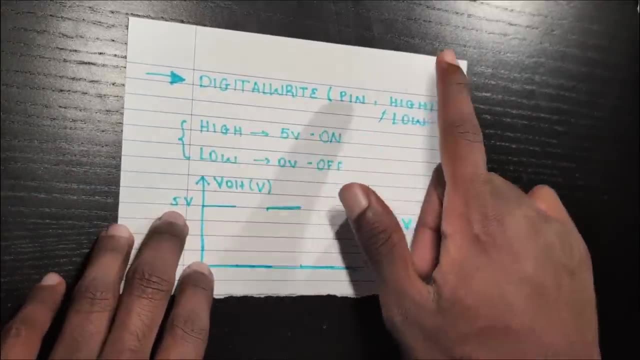 So the question still remains: why are we using integers? So, right here, let me start from something that we're familiar with. We use digital right, And then we set our pin- what pin we're going to be using- and then we set it to either high or either low. 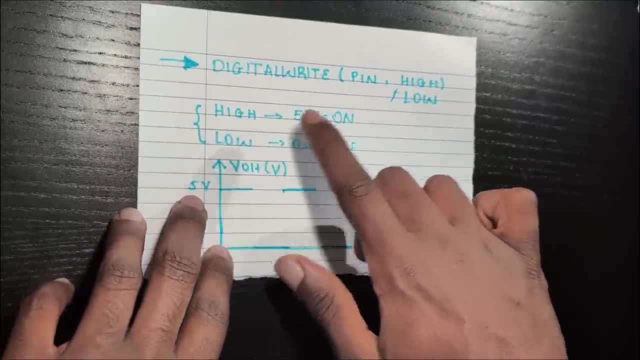 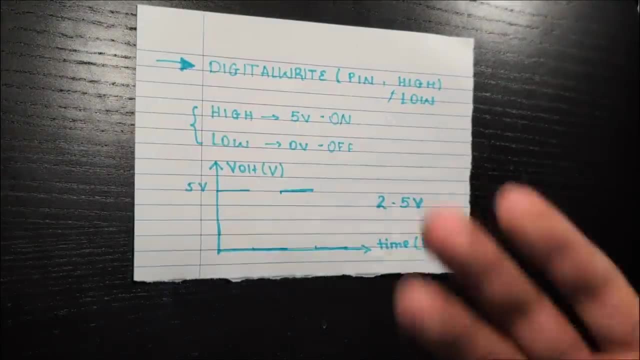 Obviously, high means five volt, which basically is on. Low means zero volt, which basically is off. It seems to be working perfectly fine. So why do we need integers to represent this? to represent high. High is represented by what? High is represented by 255.. 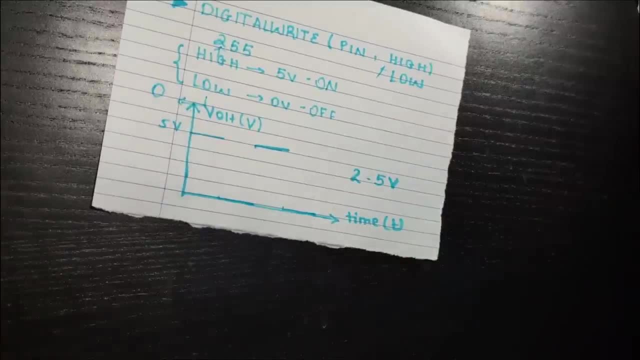 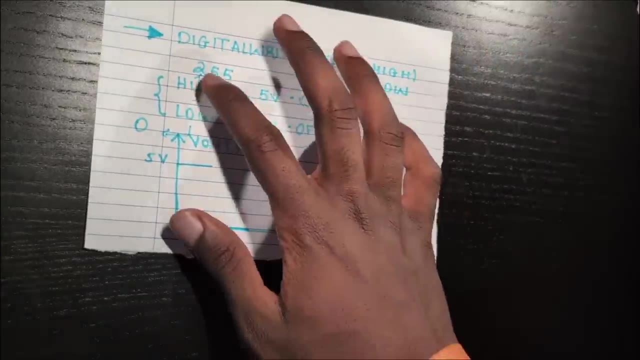 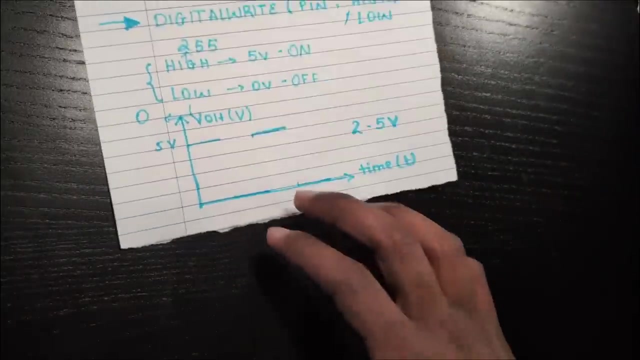 Low is represented by zero. Why do we integers to represent that? Because this gets the job done perfectly right. So the problem here is: when we're using high and low. the problem that arises is we only have two options. We cannot choose anything more than high or low. 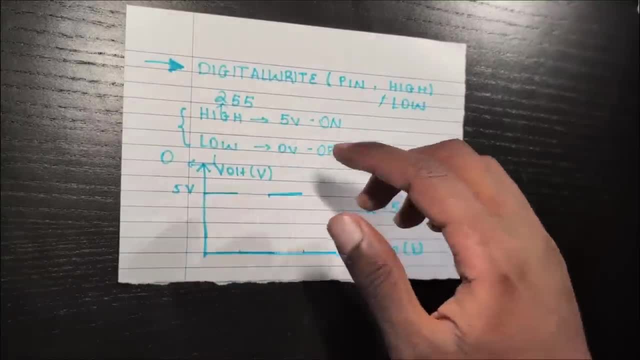 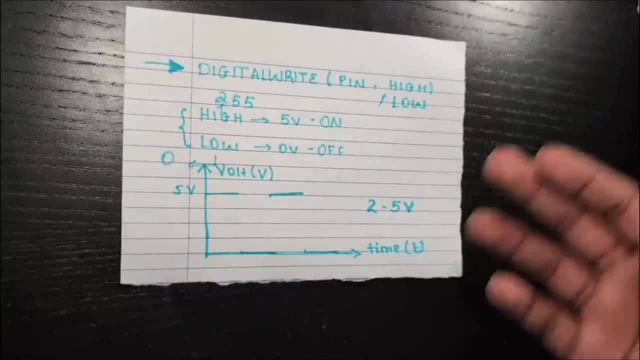 Let's say I want to set it to medium. Let's say I want to set it to well, I want it to output 2.5 volts, literally the medium, the half. What happens? I basically cannot output medium because I either I can set it to high or either I can set it to what to low. 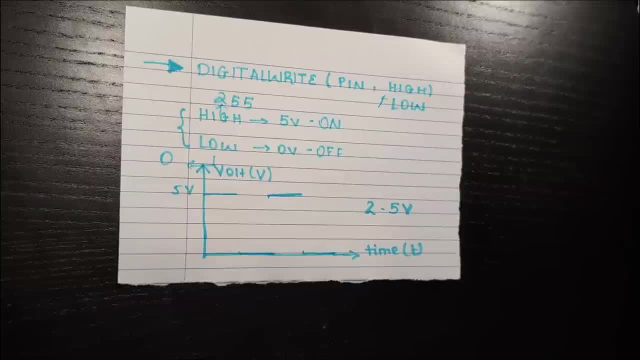 So this is where integers come in. They come really, really handy and they allow us to have intermediate values. So if I wanted to set it to medium, what do I need to do? Well, I need to do is divide 255 by what? 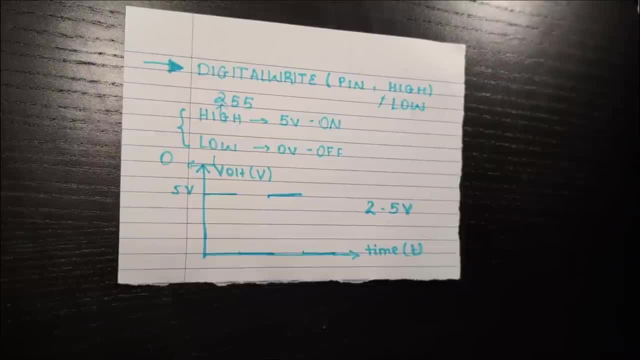 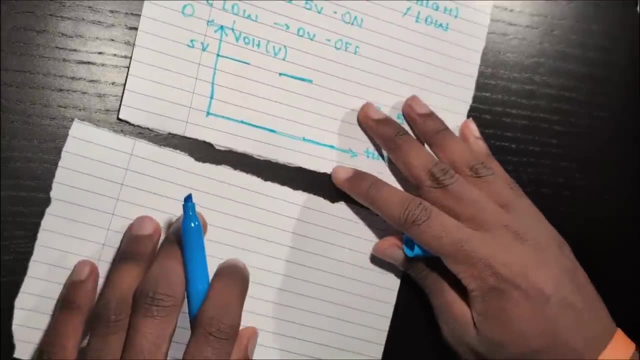 By two, basically giving me half. So let me, let me just bring a paper right here. OK, there we go. So let's say I want to do 255.. I want to. I want the half of it. 255 is what. 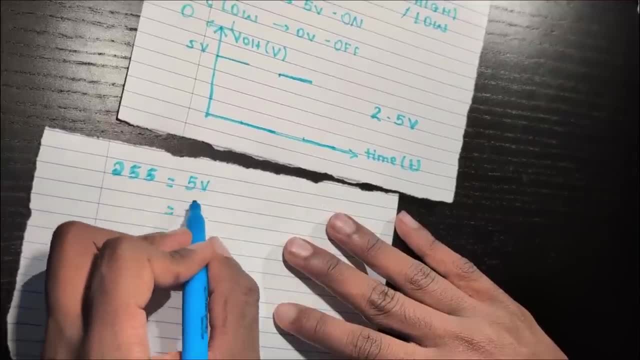 If you remember five volt, All right, I want to output half of five volt. It's going to be 2.5 volt right here. All I need to do is what I need to do: Try to find X right here. 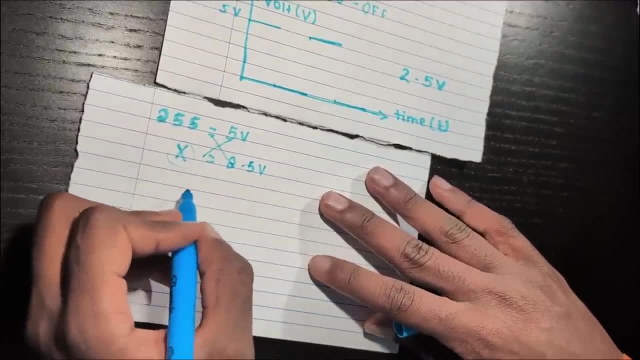 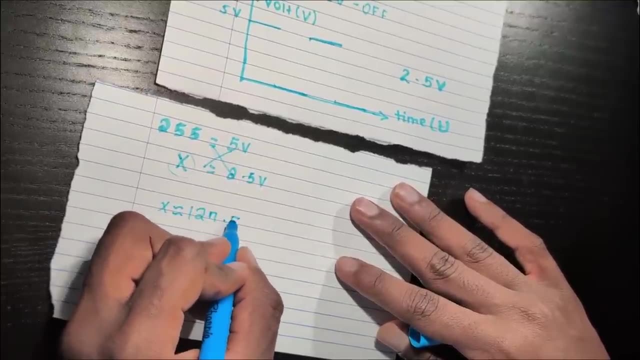 How much I should be writing Down and then do the math, And once I do it, X is going to come approximately to 127.5, which you can round up or round down, which I'm going to round up to almost 128. 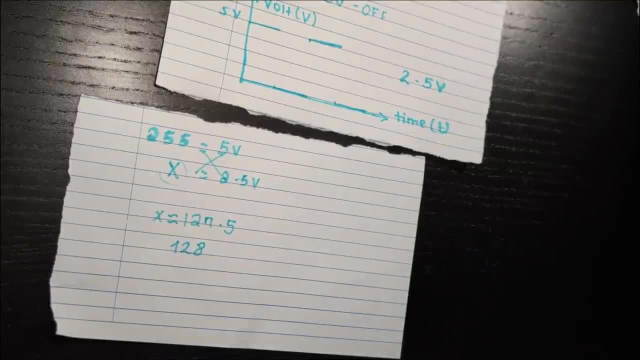 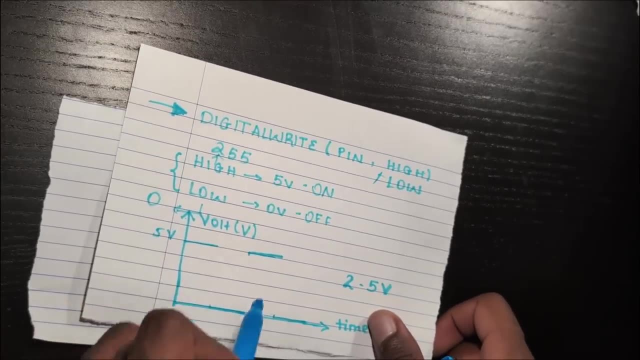 So what does integer allow us to do? Integers allow us to have intermediate values. What else Let's say I want to do is what You know what. I don't want it to be half. I want it to look. I want to do 20 percent of what. 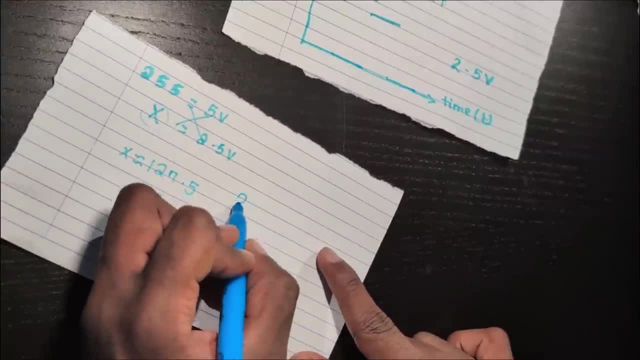 The original high that we had. I want 20 percent of it, I want 20.. I want 20 percent of five volt. I want to output 20 percent of five volt. So let's do the math right here: What's five volt? 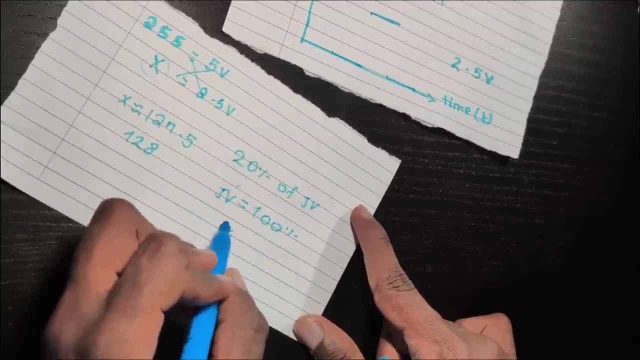 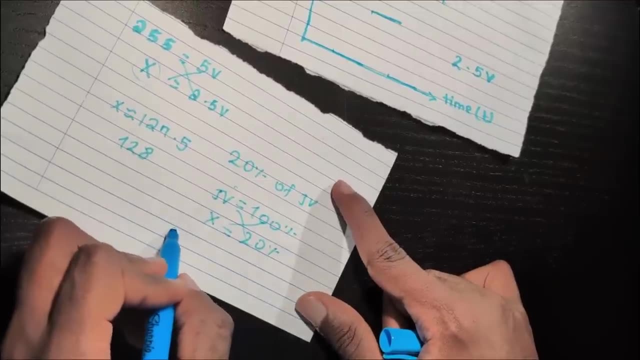 Five volt is currently 100 percent. What is 20 percent? All I need to do is find the voltage with the math right here. Keep on doing the math right here: 20.. OK, it's going to be zero point. When you do the math, 0.2 times five is going to equal to X. 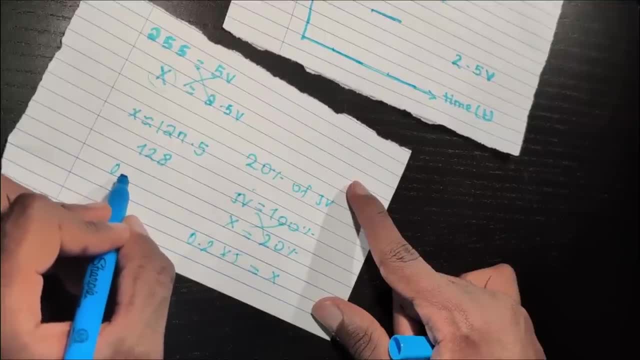 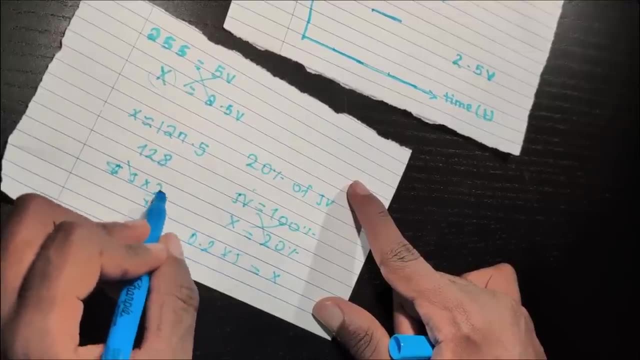 When you do the math right here, 0.2 times five. All right, So basically, what is this five? It's going to be 0.2 times two over 10.. When you do the math right here, this is going to be two over two. 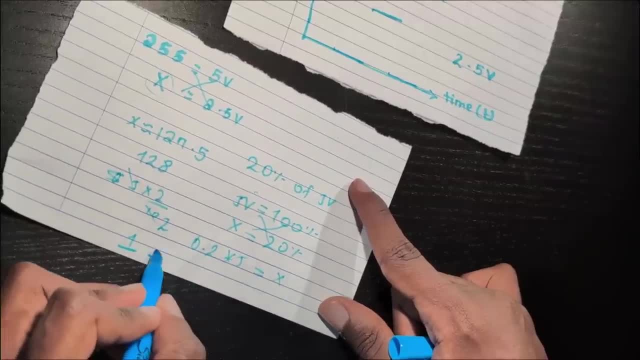 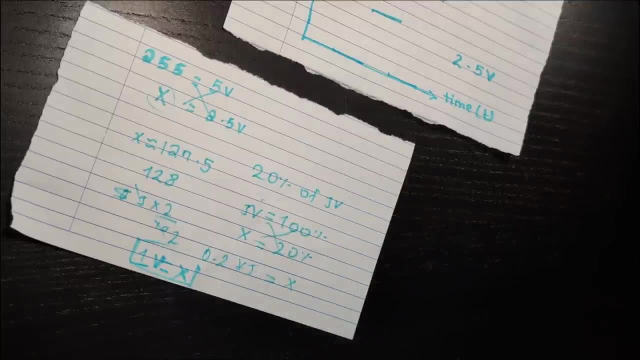 So we're going to have one, There we go. One is of course the X. Basically we're going to Apple. one volt, There we go. So basically, what it just allows to do is what we can find any value, so we can have any. 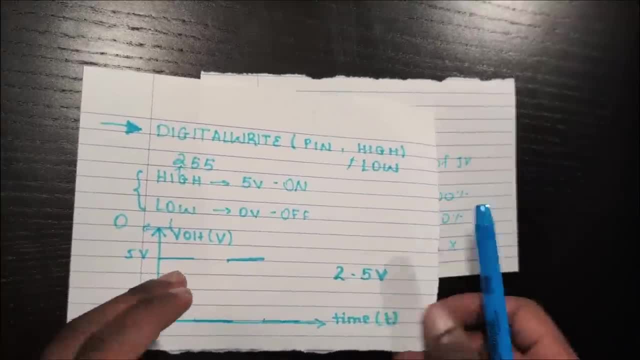 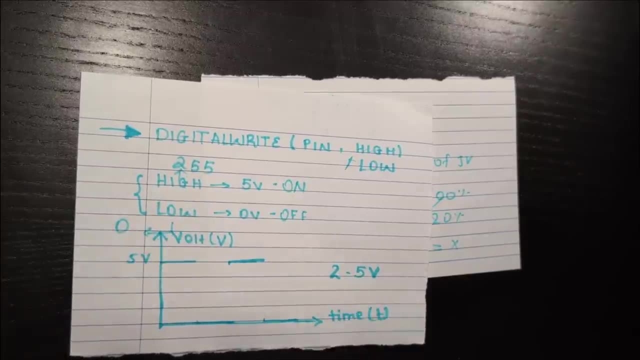 intermediate value between what? between high and low. so we can have any intermediate value between high and low, Because obviously if I had, let's say, high right here and low, let's say I write down medium For two point five volt and then I write down another name for it. 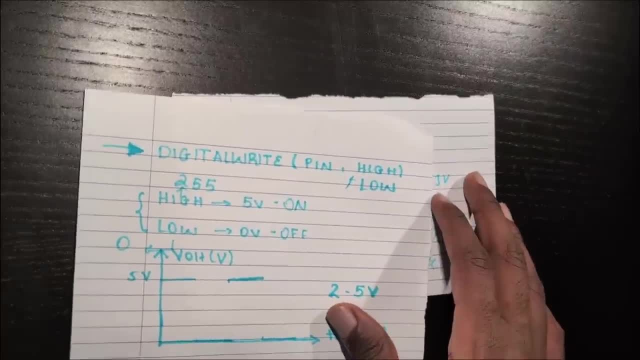 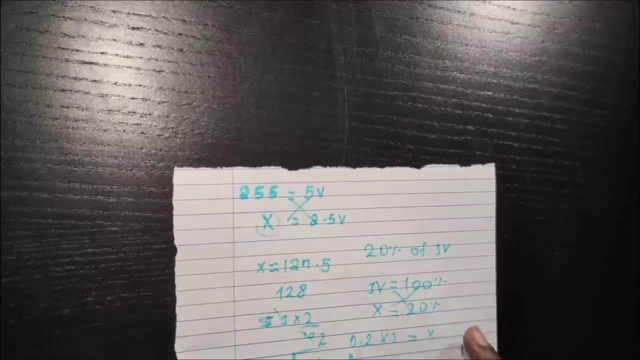 Obviously, you cannot name every instance, You cannot mean every, obviously, value of voltage. So we're going to be using integers, doing the math, And after doing the math we can do what we can: find our desired value and then output the voltage. 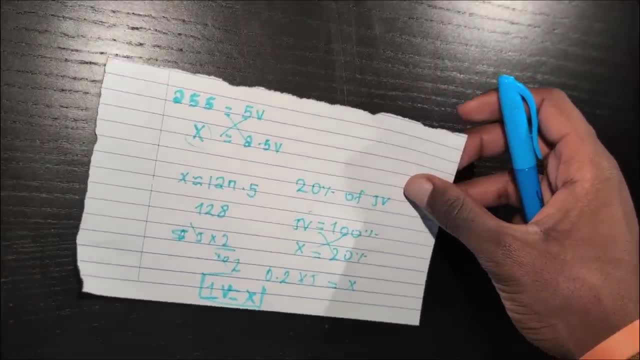 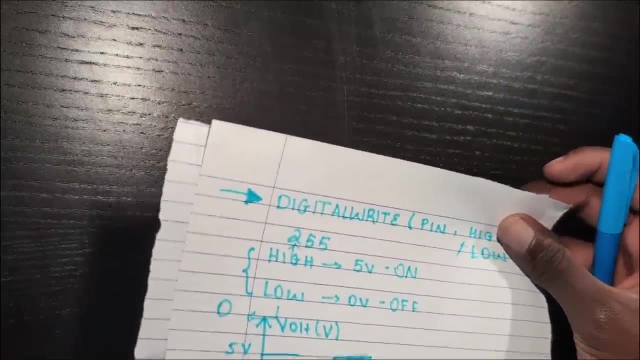 So basically we can, what we can, control the amount of voltage that's coming in to our Arduino to coming out of the Arduino. So basically what happens? Basically we can create What dimmer and what brighter light, so we can create intermediate values of light. 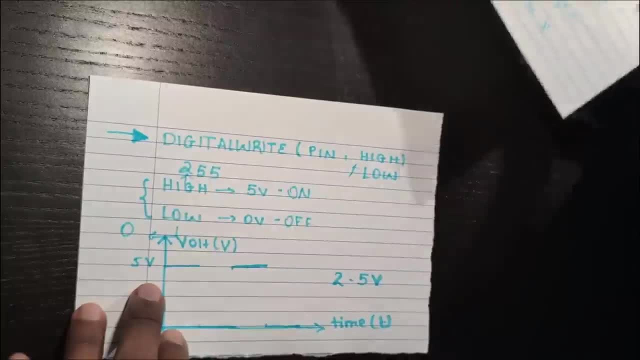 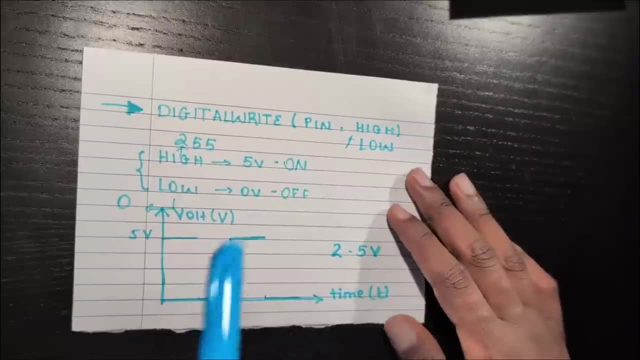 But one thing I want you guys to keep in mind is: OK, one assumption that you really really need to know is actually how it works is: it doesn't change physically. So, as I said again, when we're turning it on five volt, it's basically what it's on and zero. 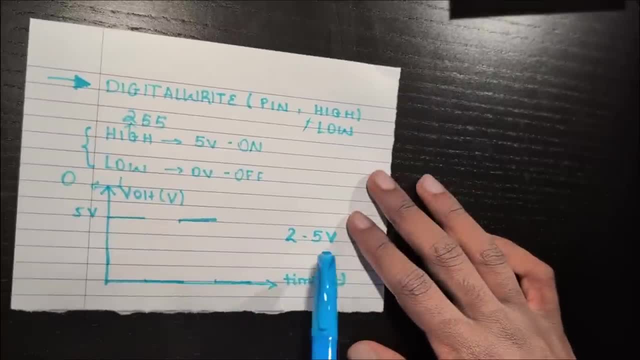 volt. It's basically up. So what happens is, let's say, you're trying to write down two point five volt, right here We're trying to what we're trying to output: Two point five volt. What Arduino does is all right. 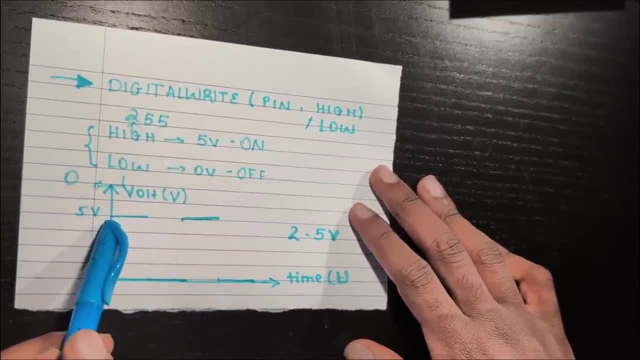 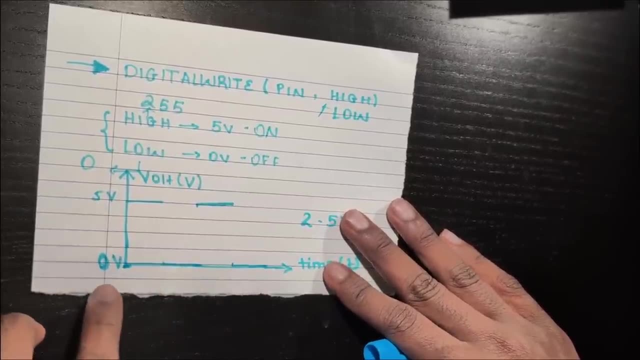 Well, Arduino does this. It turns on for half the time, for half the period of time, And then, right here, it's zero volt. You just specify it. The one on ground is zero volt, right here. So what happens is what? what happens is it turns on for half the time, turns off for half. 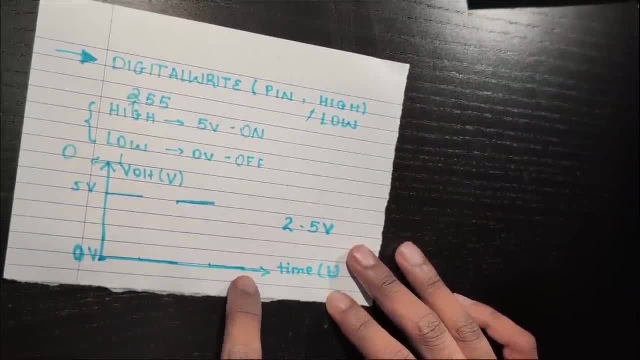 the time turns on for half the time turns off for half the time. It does it really really really fast that you cannot notice it. So for us it's going to appear as what it's going to appear: as dimmer. 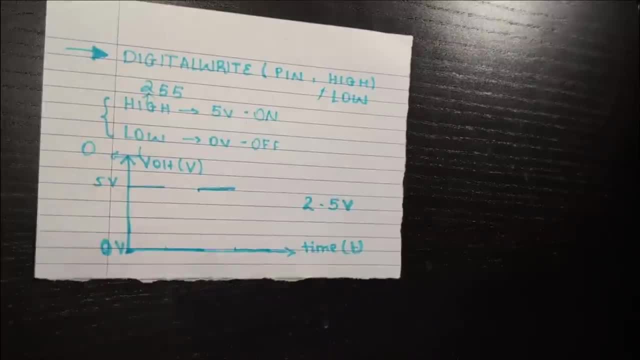 But what basically is happening is what it's basically doing: high and low, High and low, series of highs and lows. for what is doing? a series of highs and lows for again, a given amount of period of time. There we go. So that's how we act. with how much? two point five volts. 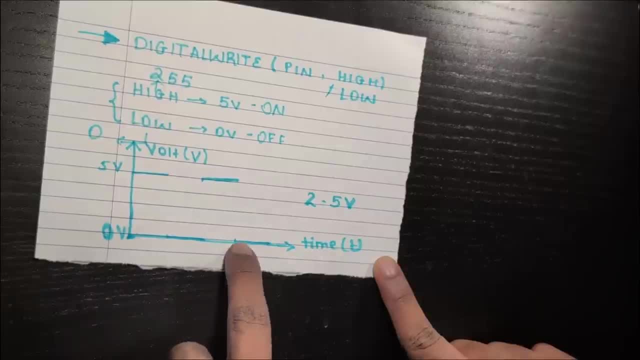 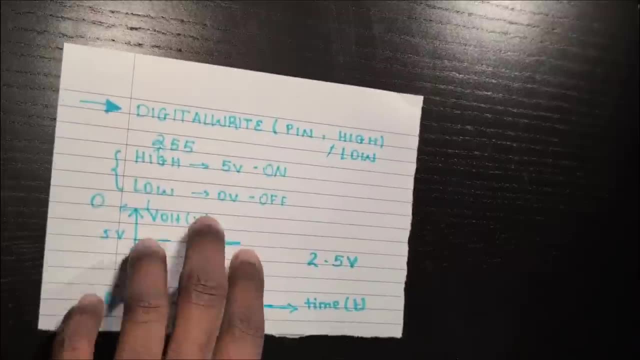 We turn off for half the time, We turn off for half the time. turn on half the time, turn off half the time. So basically we're going to have what? Two point five volts. OK, so physically the same thing is always high and low, series of five volts and zero. 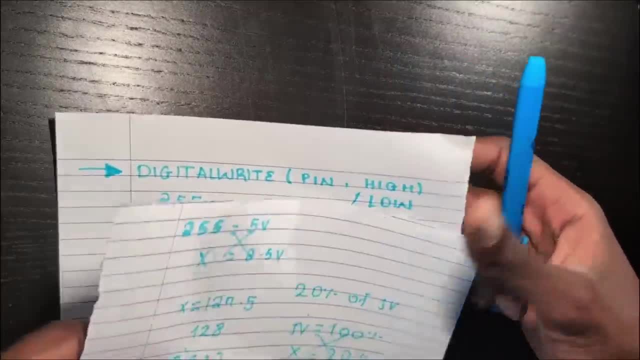 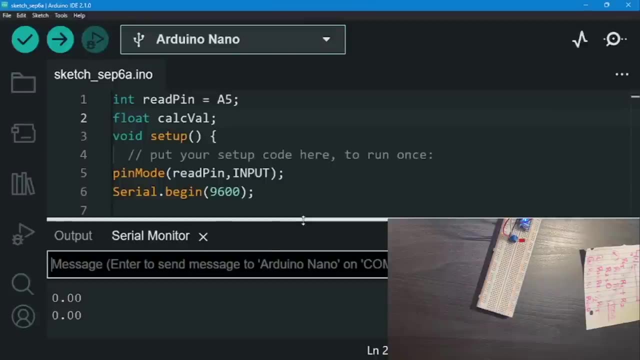 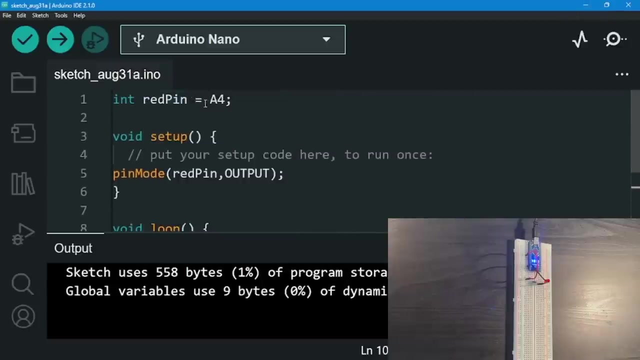 volts, But using integers allows us to do what The allows to what. They allow us to use intermediate values. All right, so before running the code, let's do a simple recap. So what we did is what we said: red pin to analog pin four, and we set it as an output. 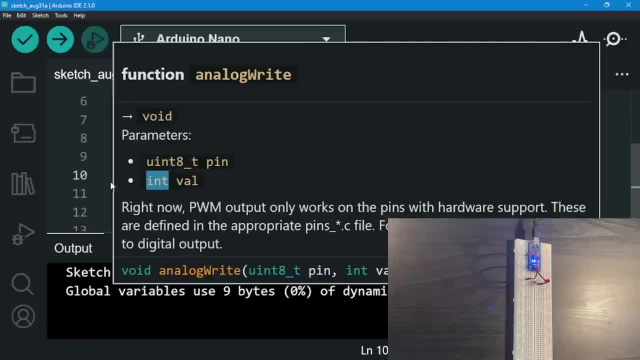 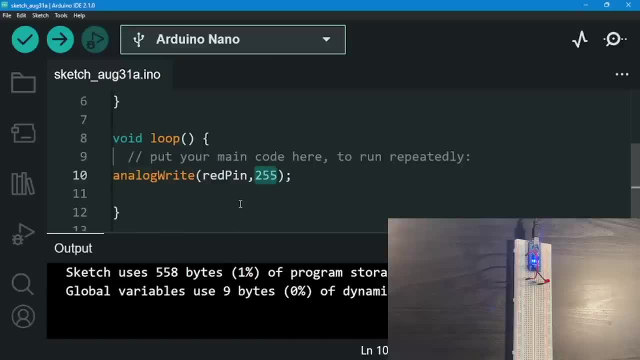 right here, a red pin, and we use the analog right command right here, analog right command right here, and we set it to a maximum value of twenty fifty five, which corresponds to five volt. All right, so let me just upload it right here and it should light up. 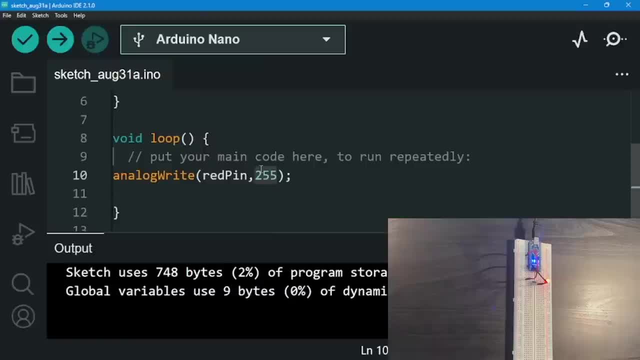 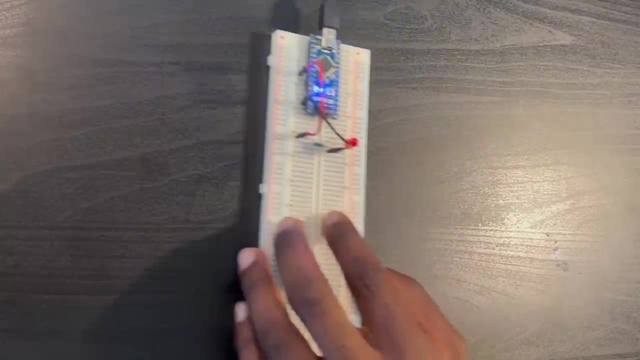 It does. OK, nice. So let me go right here and let's just say I set it to a value of forty, Just didn't notice the difference. So let's see if it goes dimmer. And when I do that, you see what happens right here. 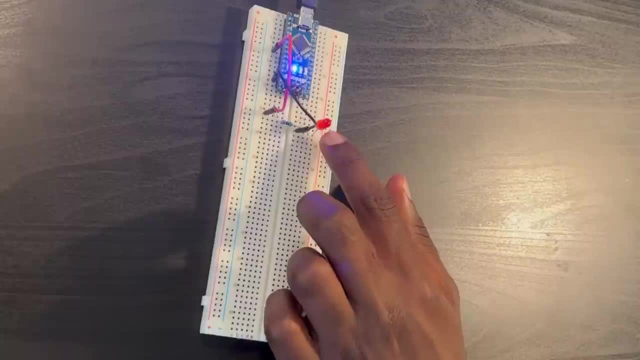 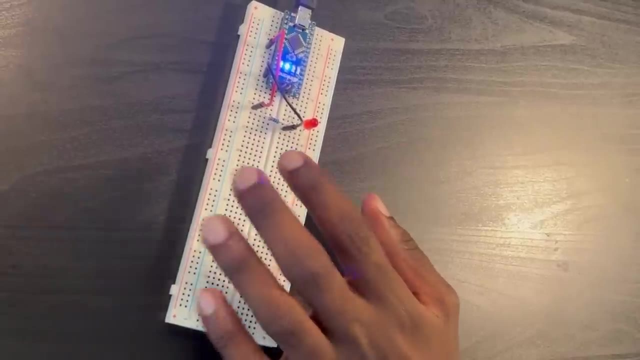 You see what happens? It does not fully turn on. So even you guys can, I'll see that it's fully turned on. It's not even turned on at all. All right, I can see that it's not turned on too. 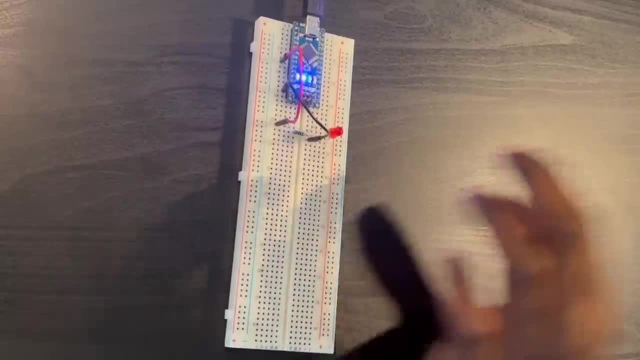 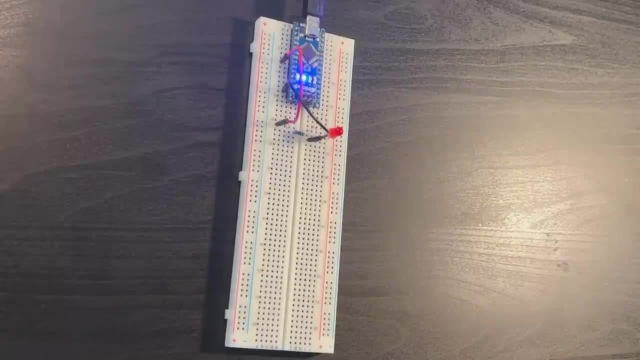 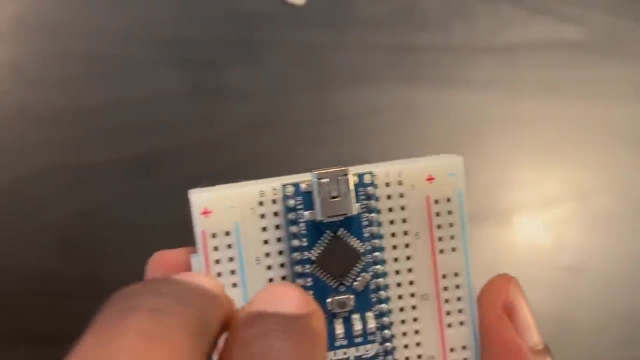 So there is an error ongoing here. So one error that I came here to fix is that what I did wrong was right here. I used analog pin four. So one thing right here- let me go closer- is that you're not supposed to use this. 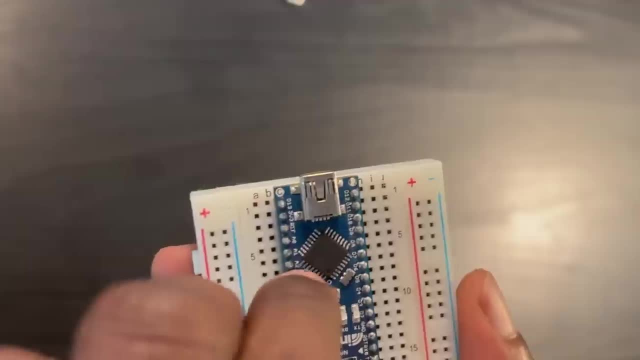 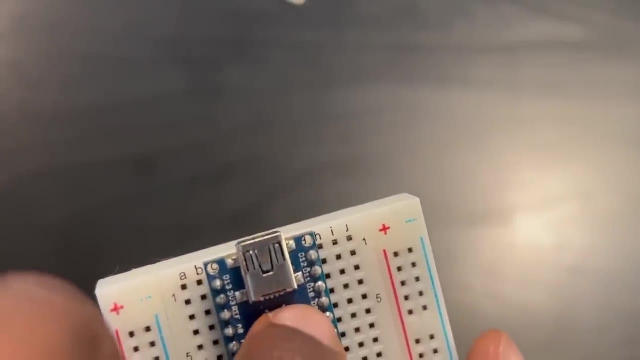 analog pins, this eight pins for this purpose. OK, We're supposed to use. Is this digital pins? right here, these digital pins that are marked with a symbol? right here? So let me go closer again for you to see it. Can you see digital pin nine right there? 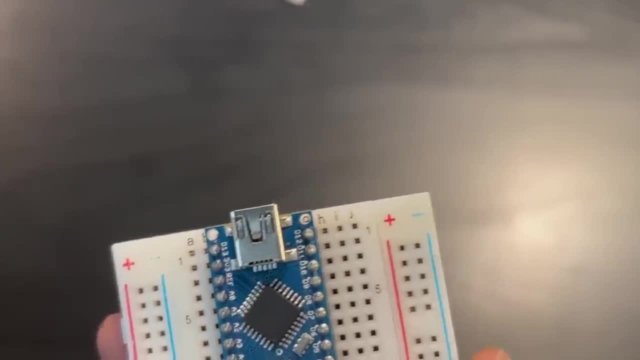 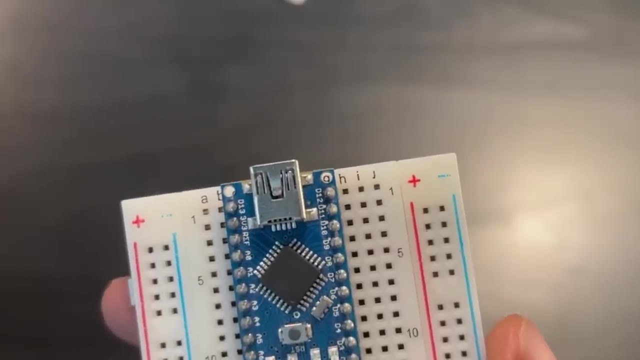 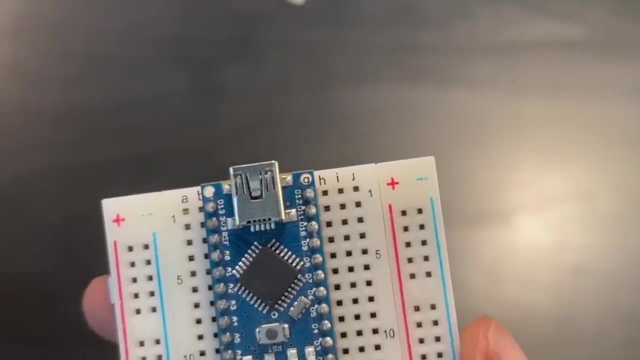 It has a dot on it, a small dot. See that. Let's compare digital pin nine to digital pin eight. If you do that, digital pin nine has a bit of a dot on the very edge. If you look at it, not only digital pin nine has a digital pin ten. 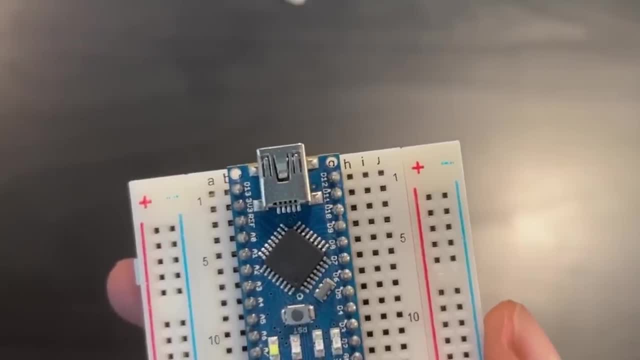 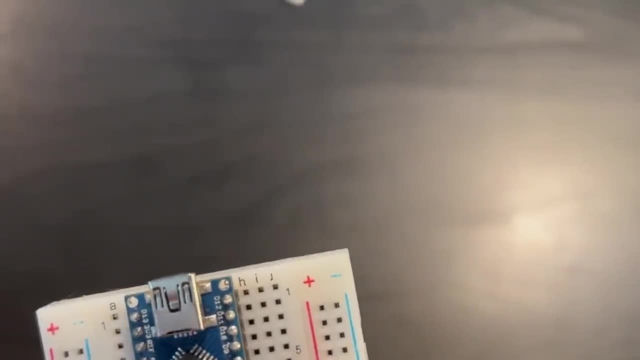 There's still pin eleven, there's still pin six, there's still pin five, and digital pin three have the dot sign on them, All right. So let me go right here, and I have to connect these digital pins that are marked with a dot or a squiggly sign. 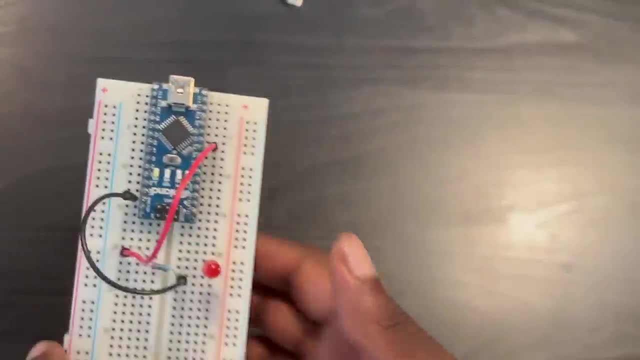 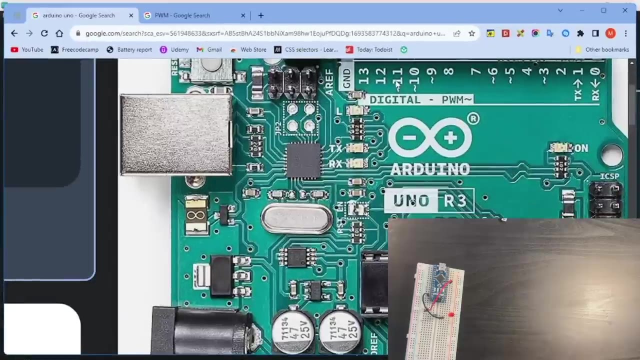 So for me it's a dot. But if you go over to my screen right now, just go over to my screen. If you go to my screen right now, what happens is there's this squiggly sign. I'm just 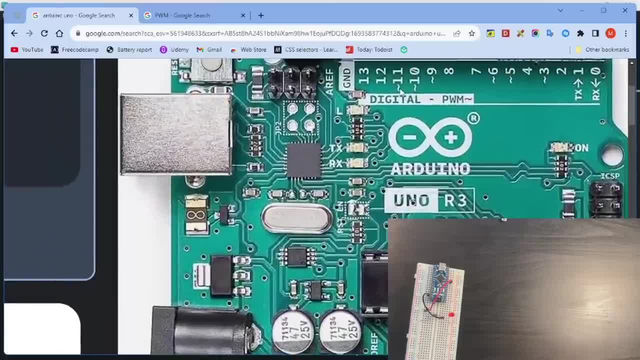 Turning on an Arduino- an image of an Arduino Uno- And if you look closely, there's this squiggly sign in front of this digital pins. So what happens again is when you're using Arduino Nano. the board that I'm currently using is an Arduino Nano. 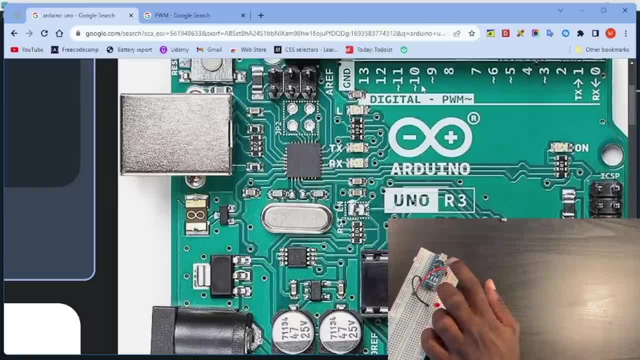 We use, we have, is what dots that mark this unique digital pins. I'm going to get to using them, All right, But when you use an Arduino Uno you have a squiggly sign, So it will vary. The sign will vary depending on. 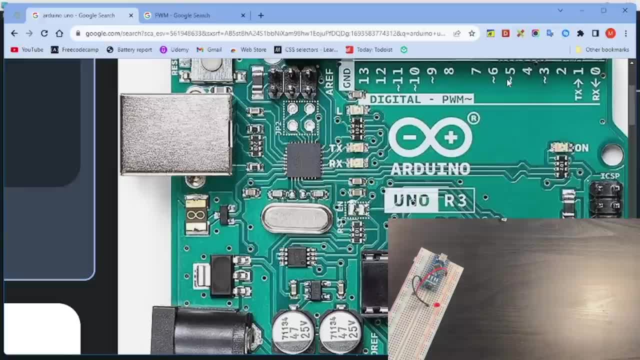 The board you have, Right, So look for if you're using any other board is look for a unique mark on your digital pins. OK, So if you look closely here, it says it supports something called PWM. OK, So PWM stands for pulse width modulation. 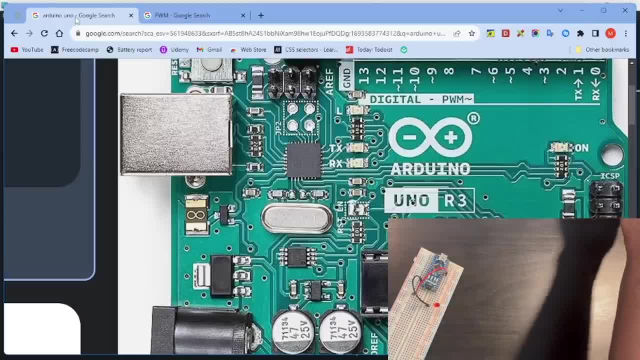 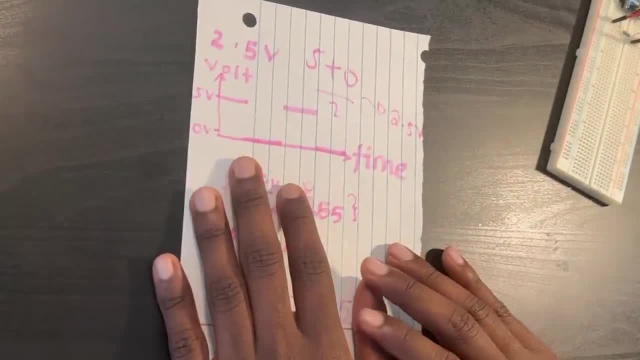 So what basically this means is, let me just explain it in a very, very simple term. All right, So before running the code, let me just, let me just make sure that you understand The signs behind it. OK, So it's quite simple. 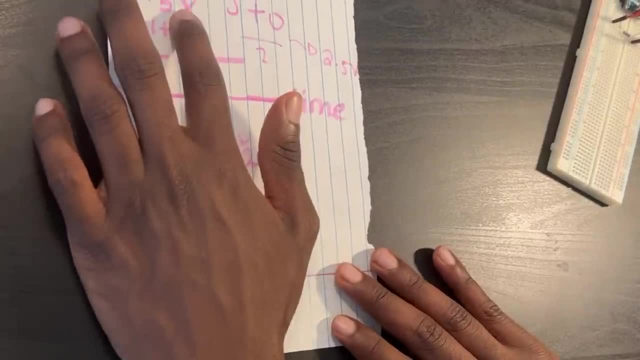 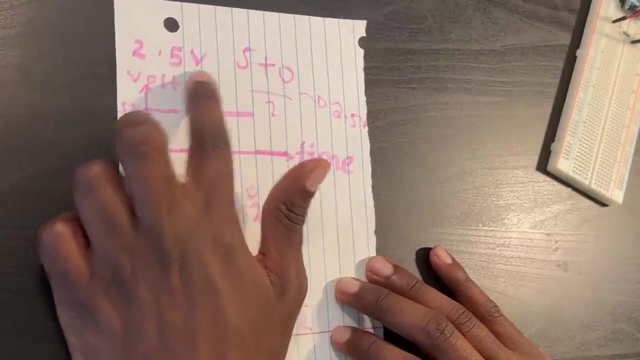 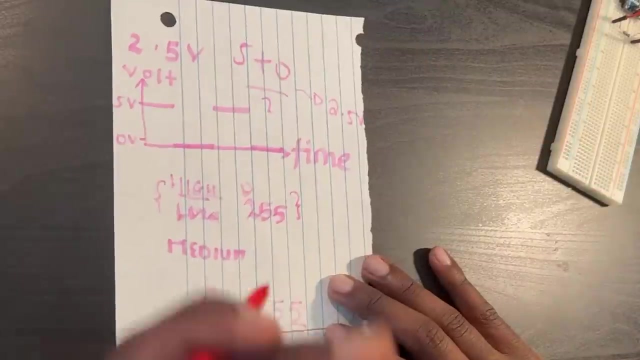 So what does this mean is, let's say, I want to turn on my, I want to turn my, my Arduino, to two point five volts. I want it to output two point five volts. All right, If I wanted to output two point five volts, let me just show you how you can do it. 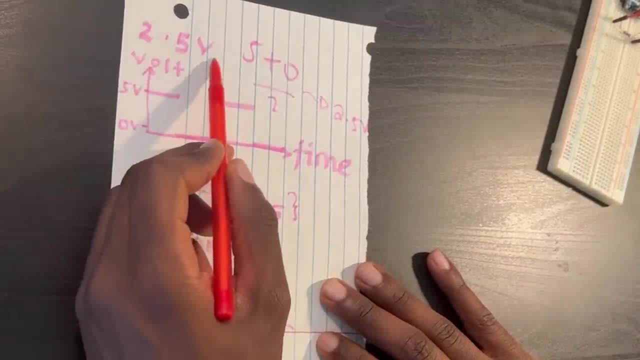 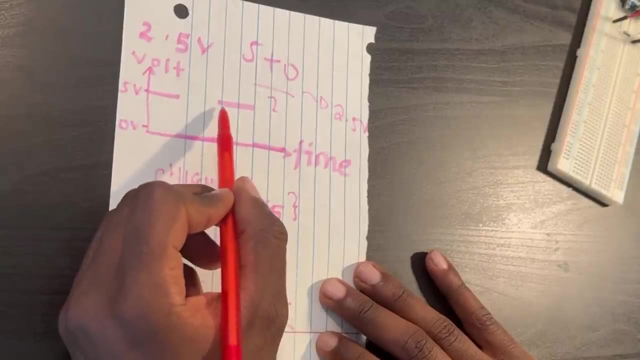 So what happens is when, let's say, an Arduino outputs two point five volts, what happens is it goes to five volt Half of the time And it goes to zero volt half the time. It goes to two five volt half the time and it goes to zero volt half the time. 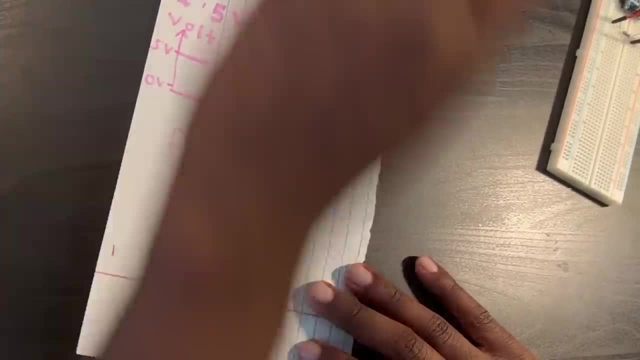 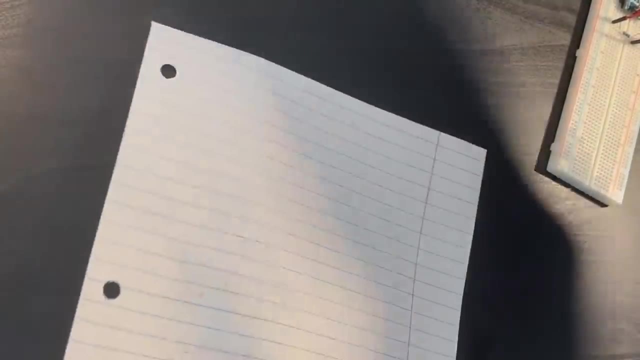 Let's say I want to turn on to. let's say I want to turn it on, Let me bring another paper. Let's say I want to turn it on to one, All right. So let's say I want to turn it on to one volt and just turn on. 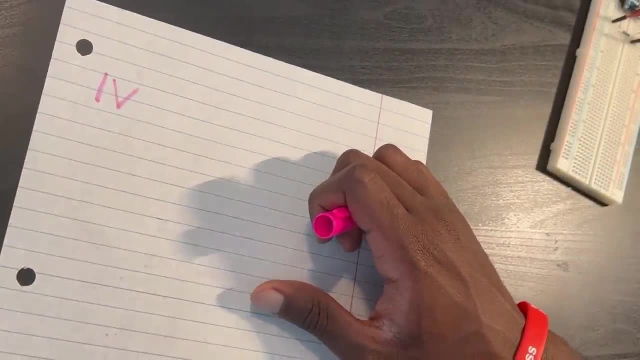 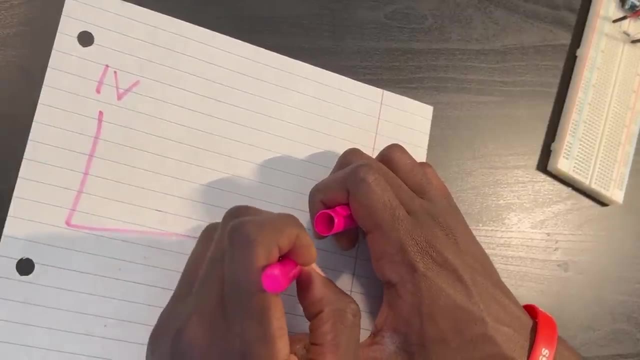 There we go. Let's say I want to turn on to one volt. OK, How do I do that? All I need to do is just again draw the graph of volt versus time. It's this time right here with the time volt versus time graph. 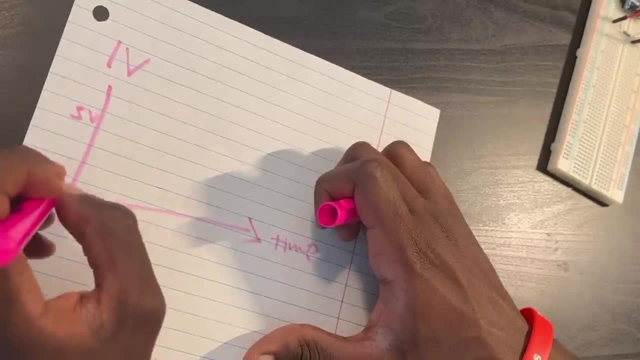 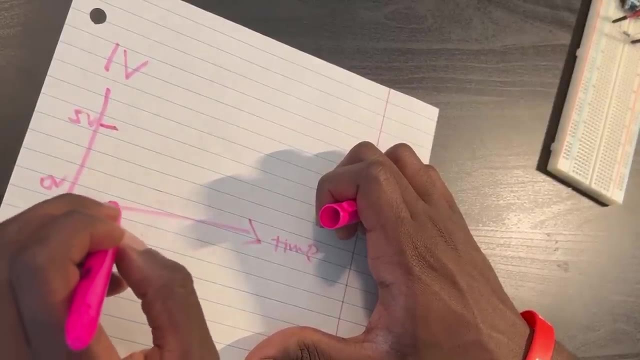 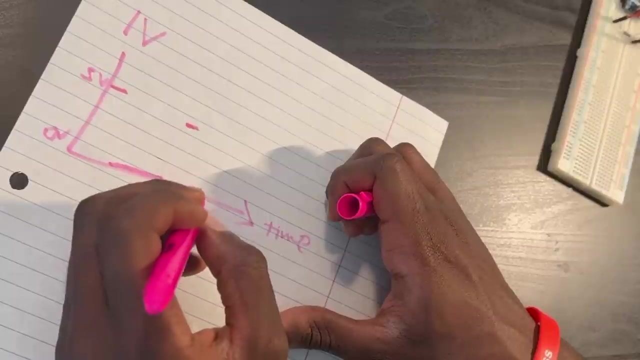 So what happens is it turns on. it's five volts right here and zero volts right here. So what happens is it what it turns on for a very short period of time, It turns off for a long period of time. You see that turns on for a long short period of time, again for five volts for a very short period of time, turns on for a long. 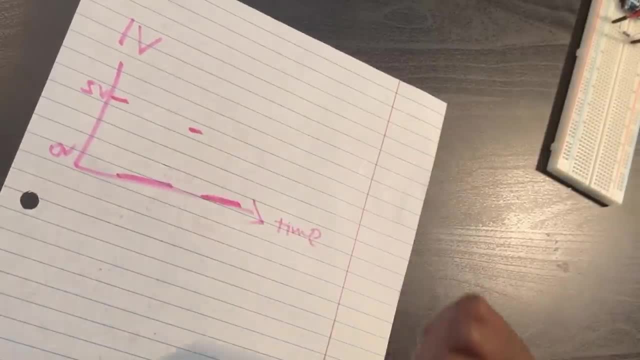 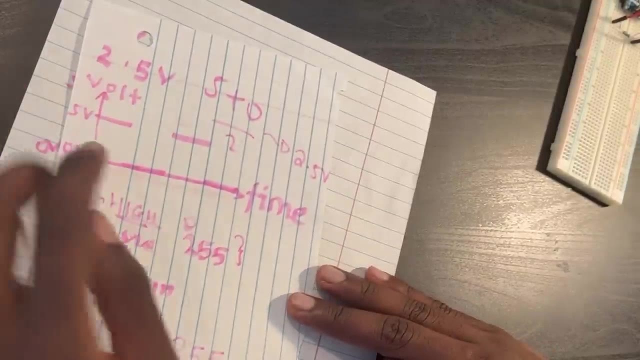 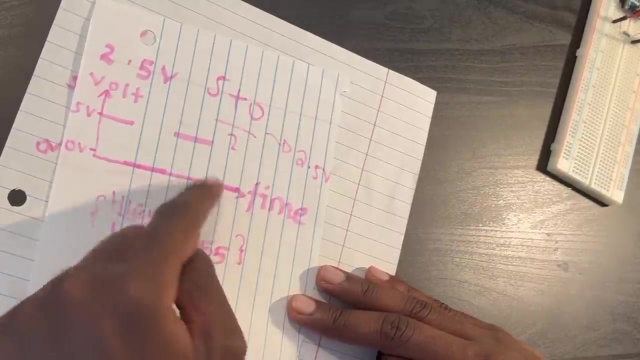 There's up for a for a long period of time. okay, that's just a rough sketch of how one volt will look like. when it comes to 2.5 volt, what happens again is what? half the time it turns on, time turns off. half the time turns on, half the time it turns off. so we achieve this voltage. how do we do it? 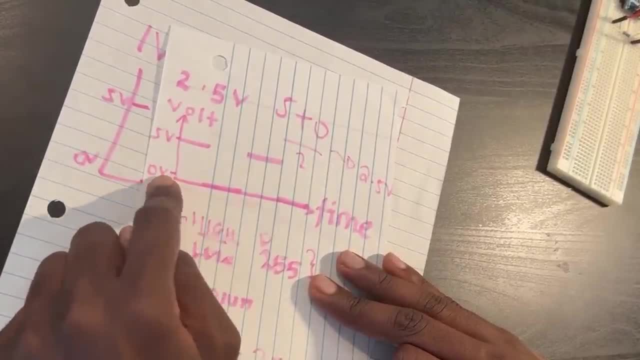 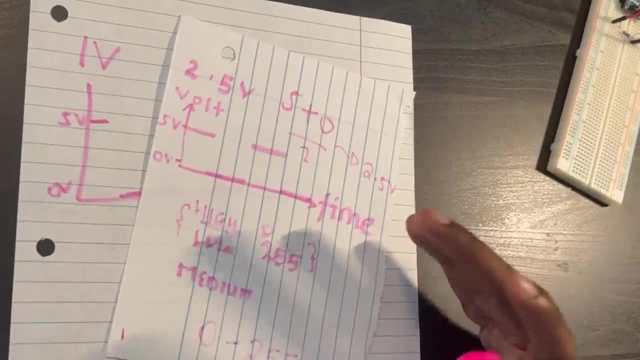 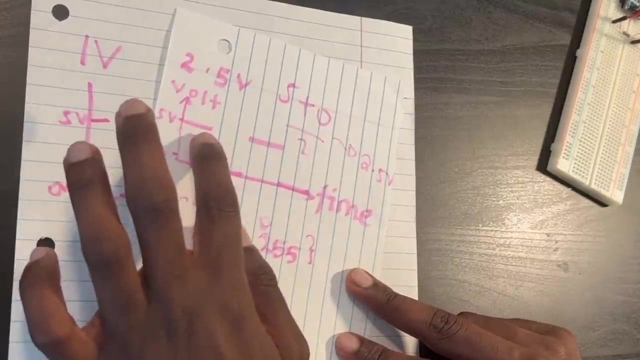 we use the two ends- five volt and zero volt- and we what? we fluctuate between them, so we change between them. okay, that's the science behind it. and one thing i want you guys to know is this: it happens at very fast speed that we can't notice it turning on and off, so we don't see it. 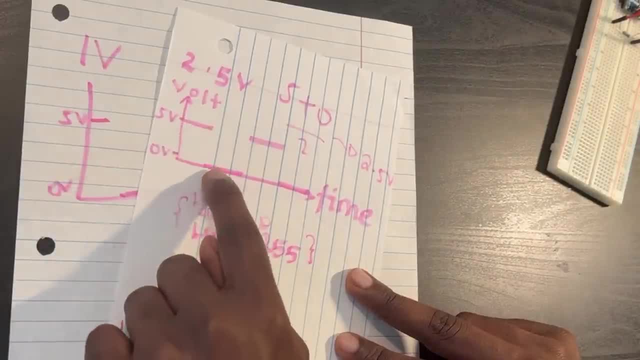 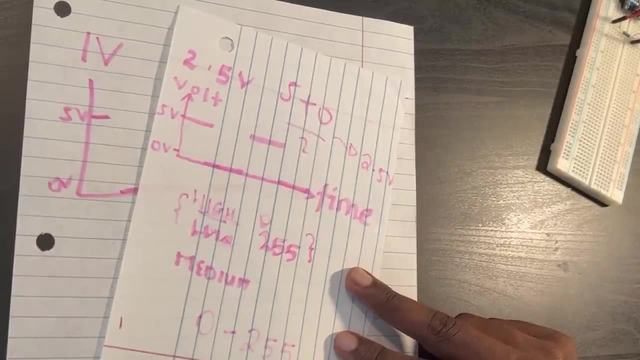 turning off and like for like five volt for half of the time and turning off for half the time. it happens at very, very fast speeds- i'm talking milliseconds- that our eyes cannot notice the difference. okay, so for us it's going to appear as a dimmer light, even though it's turning on and off. 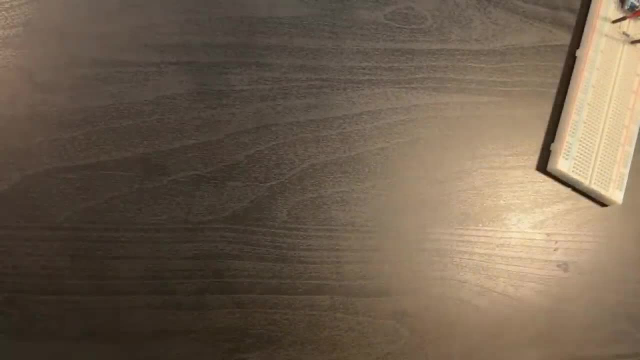 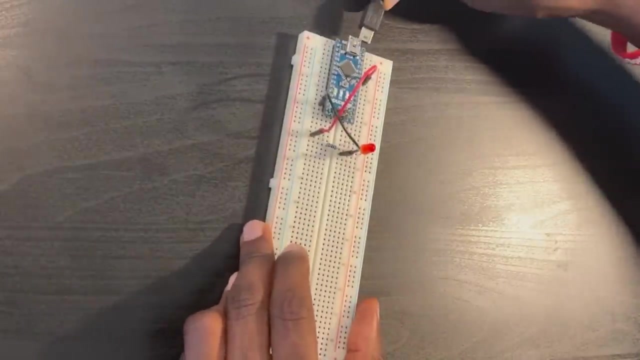 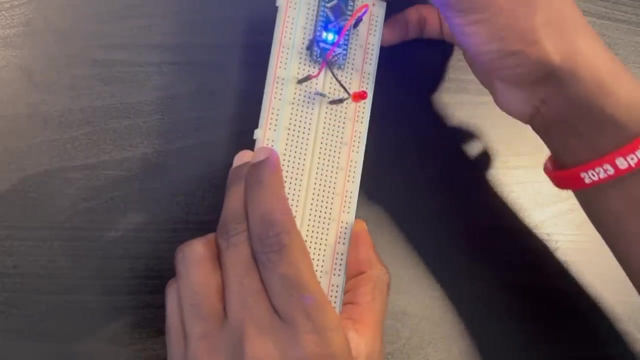 on and off at very, very fast speeds. so let's go to our code and let's write it down to actually see what happens. so let me again plug my arduino right here, okay. so right here, let me actually actually, instead of plugging it, what i 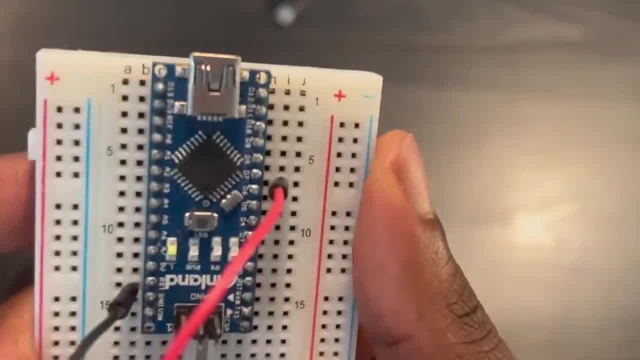 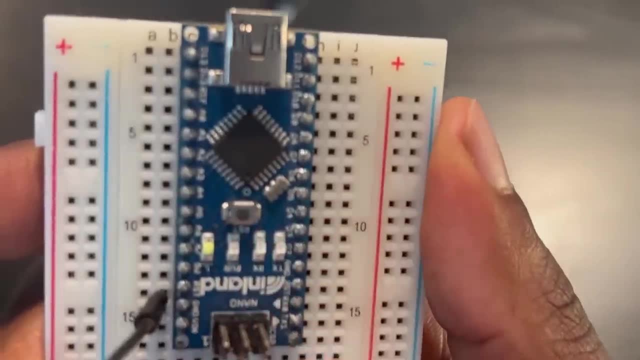 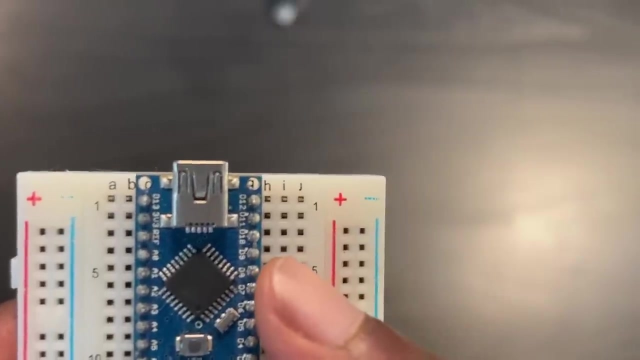 should do is let me bring it closer to you guys. so right here, one thing you can notice is we can use those squiggly signed. can you look at it, those pins again with the squiggly sign on them? so in this case, digital pin 10 has a squiggly sign. digital pin 9 has a squiggly sign. let's just 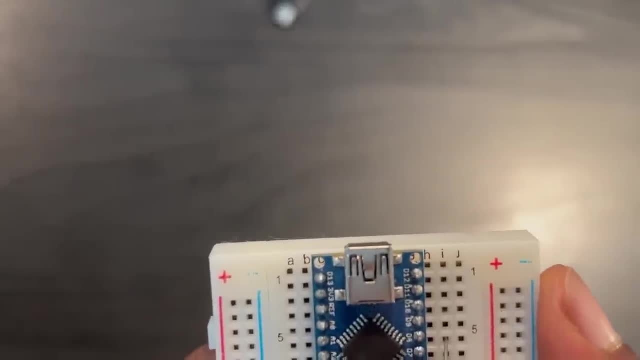 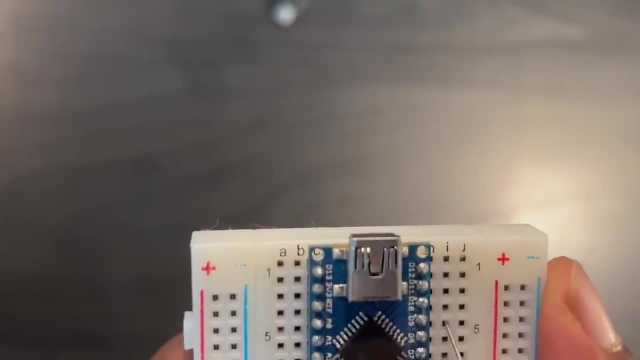 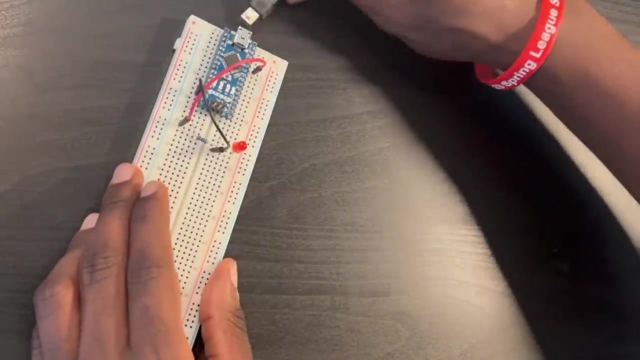 use digital pin 9 right here, okay. so use one of those pins that have a squiggly sign or a dot in front of them. so there's still pin 9. i have to go right here, all right. so i connected it to digital pin 9 and again, it's a simple led circuit, so let me connect my arduino board right here. 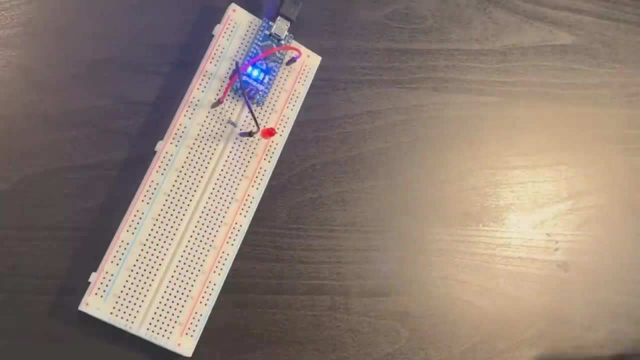 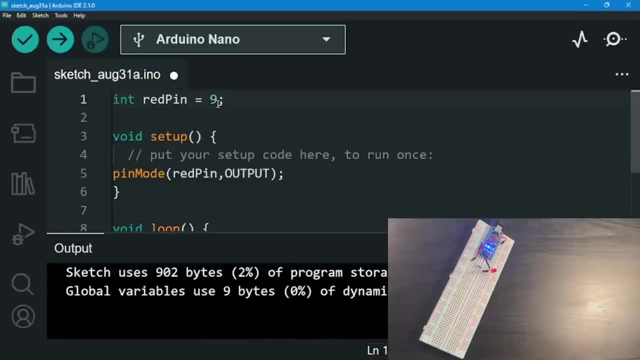 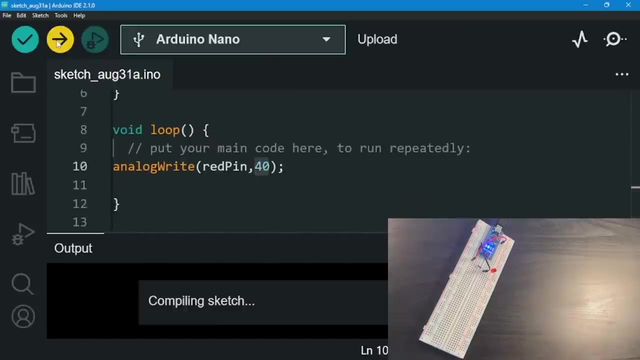 okay, let's go back to our code. let me go back to my screen right here. all right, so i'm going to say: is what pin 9? okay, then i set pin right, put as output and pin to 40. okay, so let me just upload it right here. 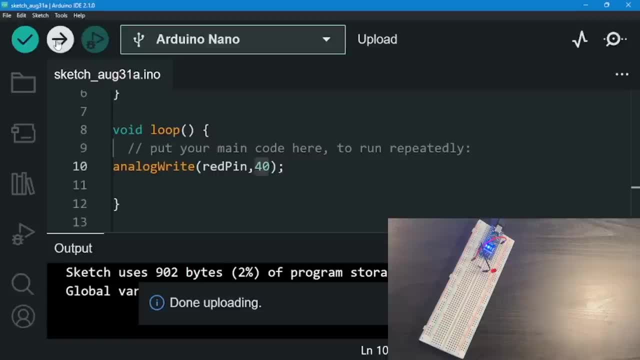 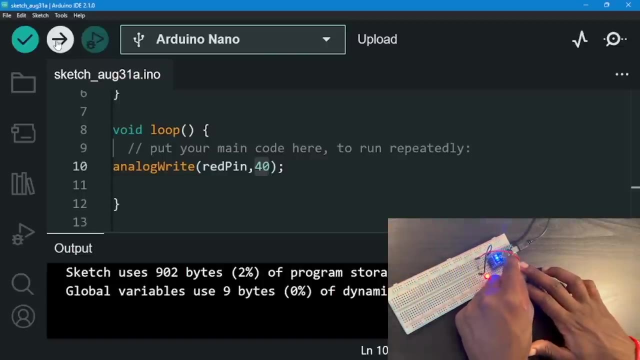 i uploaded it. it's not even fully turning on. maybe might be the resistor right here. it's not the resistor. am i correct with the pin? i might. i think i'm doubting that. okay, i got it to pin 8.. now i'm correct with the pin. it's pin 9 is right. 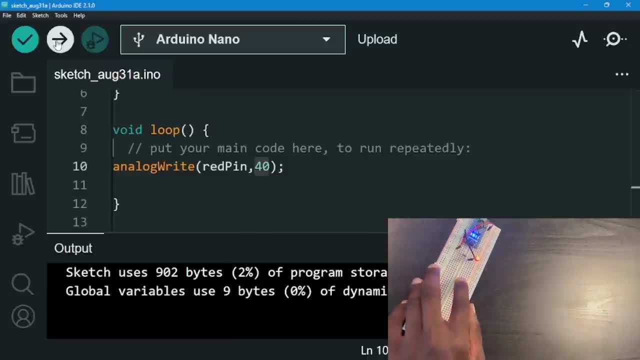 here. oh, there we go. we have a dimmer light. i don't know you might notice or not. so what i'm going to do is, uh, to notice it is, let's go to my screen and let's write some PED enforcement code for so that you guys can actually notice the difference between a value of 40 and a value of 255. so let 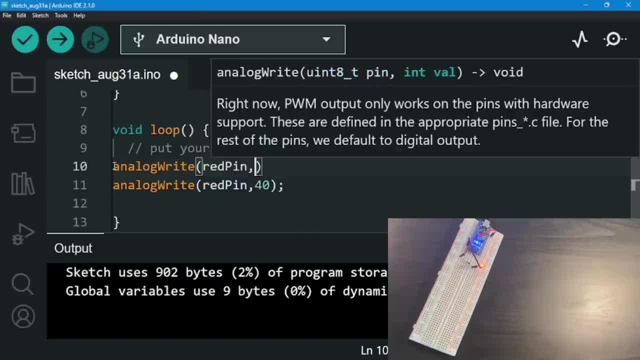 me just say: analog, write red pin and set it to 255. okay, then we're going to set it down right here. so i'm going to go ahead and prospect actually a Red Pin to the red pin setting and then i'm going to push my knob to actually set it down. alright, so i'm going to go ahead and connect it here, all right. 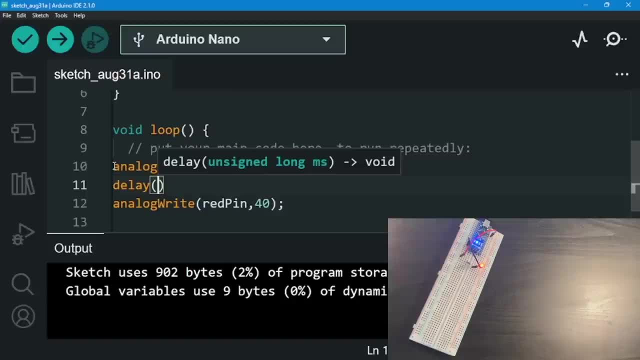 then i'm going to put in some extraaste here, then I'm going to go ahead and Popeye, probably a communicate over here- I'm set a delay again. delay function lets us put delay for the amount of millisecond. so right here I'm gonna set it for 1000 milliseconds, which basically means a. 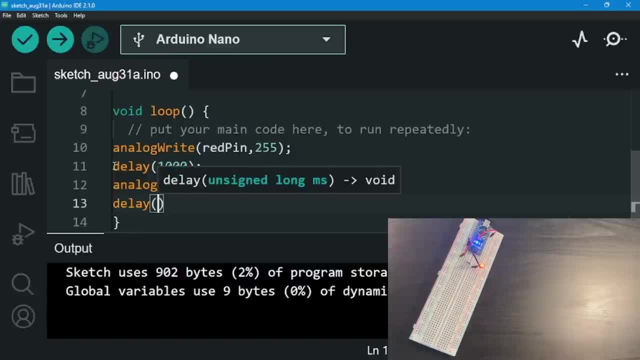 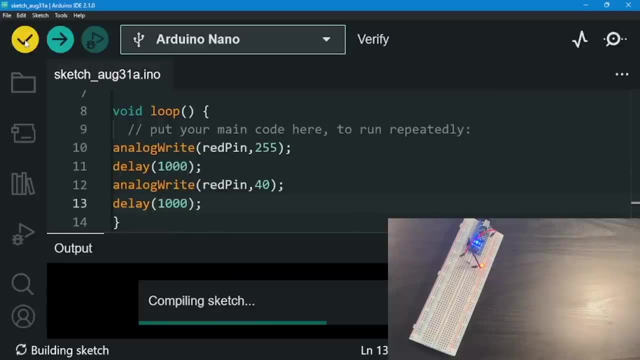 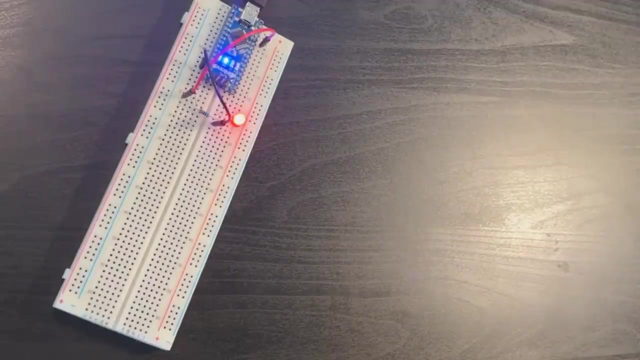 second: all right, okay, so you can see the difference. delay again 1000. so let me just run this again. so let me verify this. everything's running right and smooth, all right, and let me upload it, okay, all right, can you see it? it's going brighter and then dimmer, brighter and dimmer, brighter and dimmer. so what I'm? 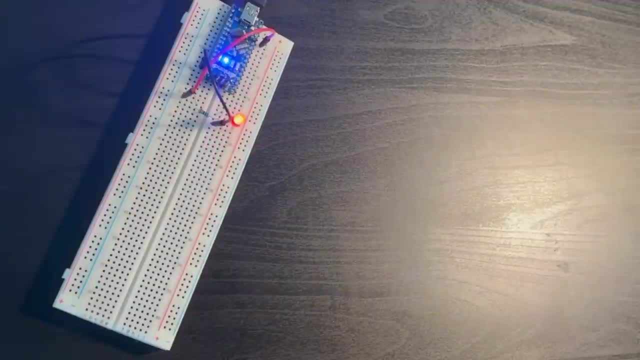 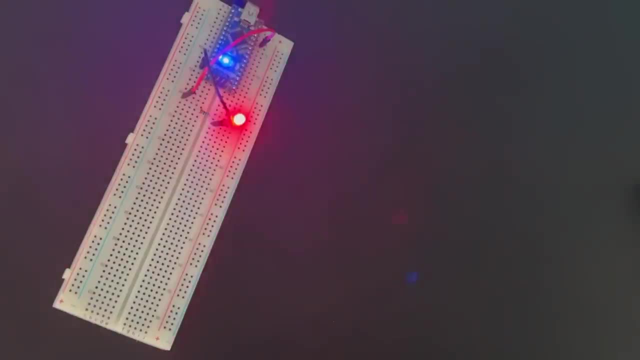 gonna do is turn off the light right here so you can see it way better. okay, let me just turn off both the lights on the spot. you'll see it better. now. it's going brighter and dimmer. obviously, the brighter is 255, while the dimmer is. 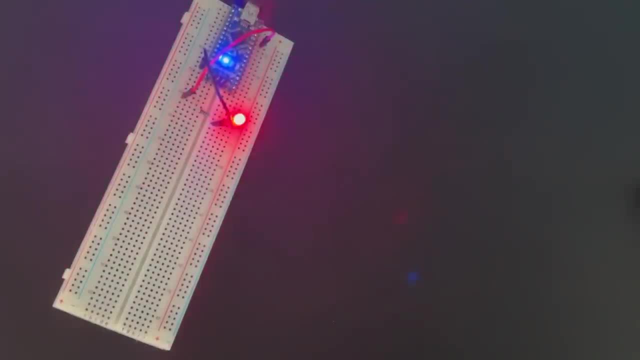 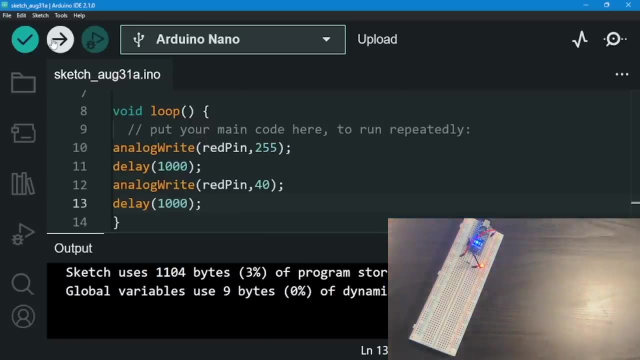 obviously the night number 40, okay, so let me just go back to our light right here. turn off, turn on both lights, so so we've seen how to pulse width modulation right here works. okay, so I'm using what PWM, all right? all right, so I'm using this pit, so one. 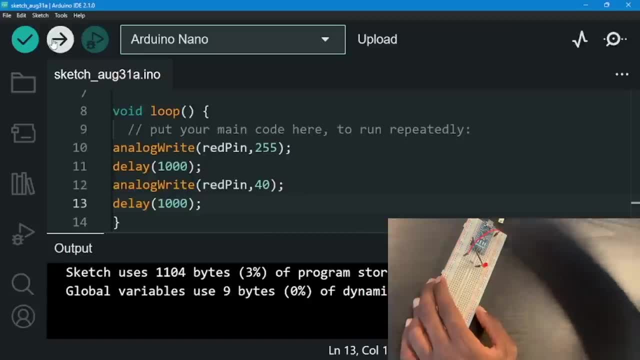 confusion that happens is what I see most often- is all right. what are again this pins? are the analog pins, the ones that are marked with, just with a D pin and then a number next to them and that have again a dot or a squiggly sign? are the analog pin or are they digital pin? 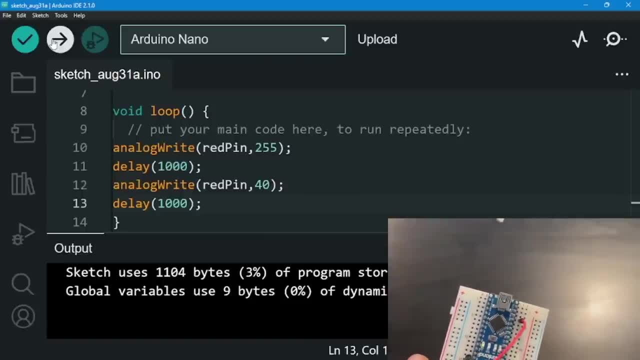 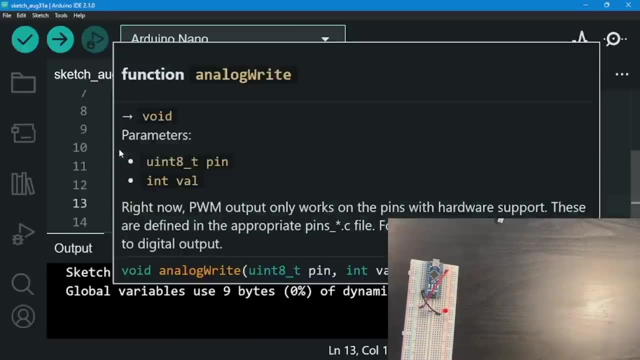 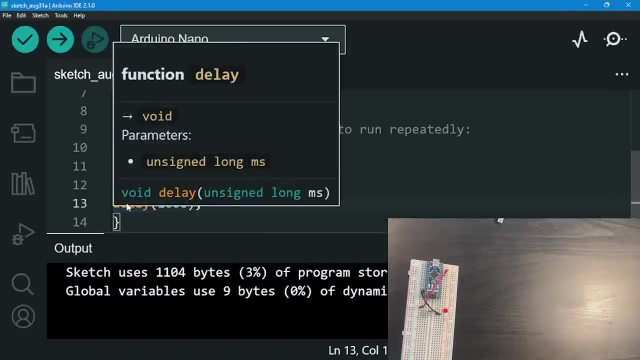 because if you again look at the code right here, we're using analog right. so if you look at the code right here, let me just highlight it again- if you use the code right here, we're using what? using the command analog right. oh my god, this is getting annoying Jesus. 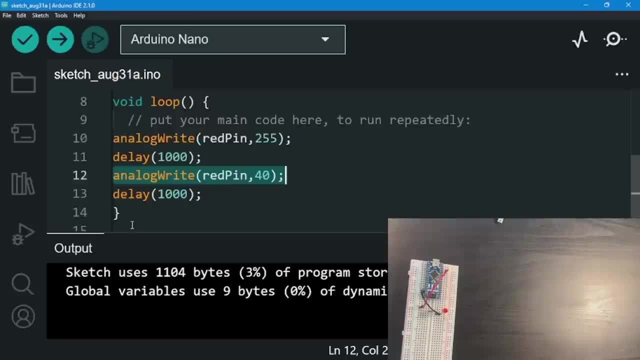 go right here: analog right, it's going to analog right. but also one thing you notice right here is what it's marked with the D, which makes it a digital pin. so maybe wondering: is this a digital pin or an analog pin? so one thing you need to understand here is the ones that are marked with a, with a dot or a squiggly. 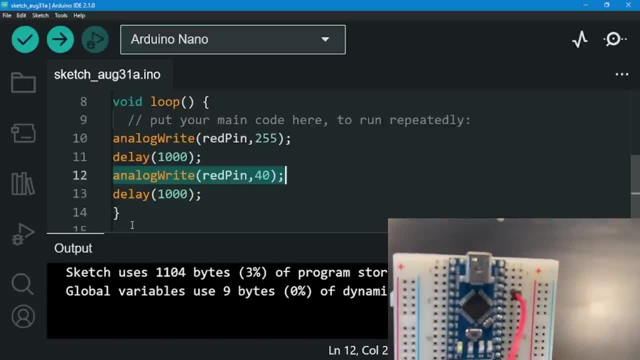 sign these special digital pins. I'll call them special digital pins. what they are is they're both okay, so they're digital pins. they're also analog pins. right here, when we use the analog right command, we use them as what? as an analog pin. okay, so we use them as analog pins. and also one thing you need to keep in mind is we 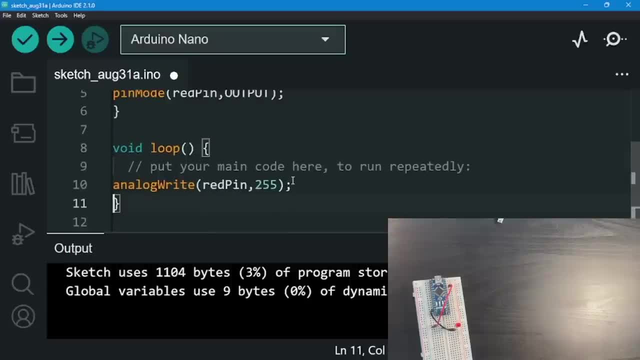 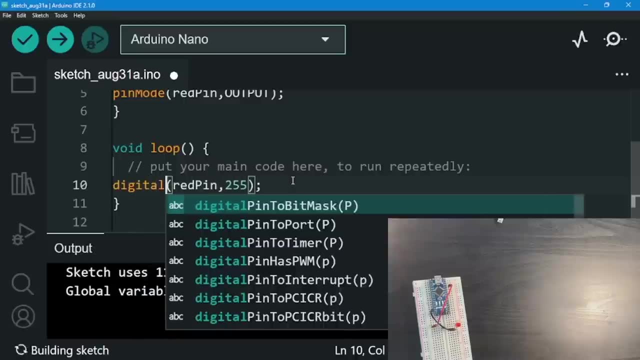 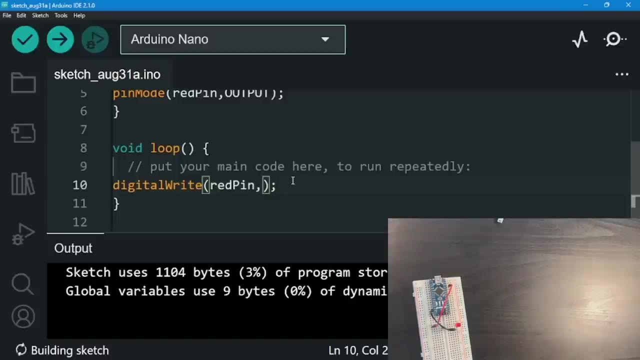 can also use them as digital pins. so let me just turn off all this code right here. if I just say this again: not changing the, not changing the pin, right here I'm gonna say: is digital pin right? there's still right right here. and again, when we use this command, we only can say high or low, we cannot put a. 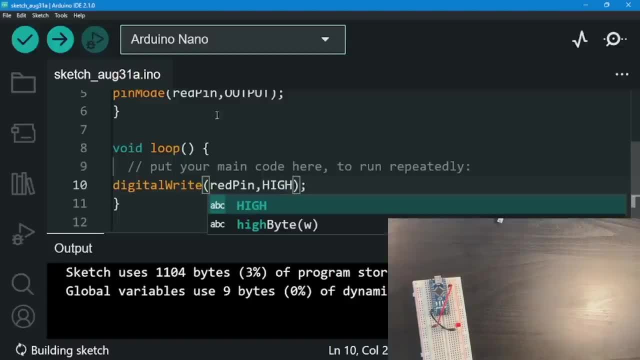 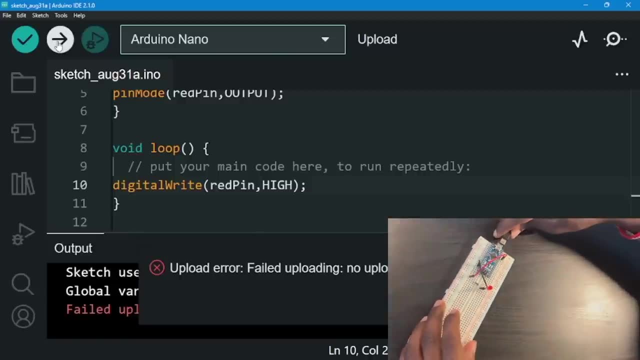 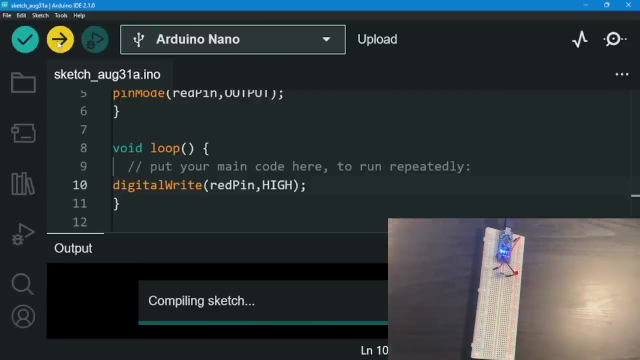 number here I'm just gonna say hi, okay, so let me upload it right now as it is, just upload it on the spot. and again, let me connect my Arduino right here. I forgot to connect my Arduino. you know I can't upload it because I did not connect my. 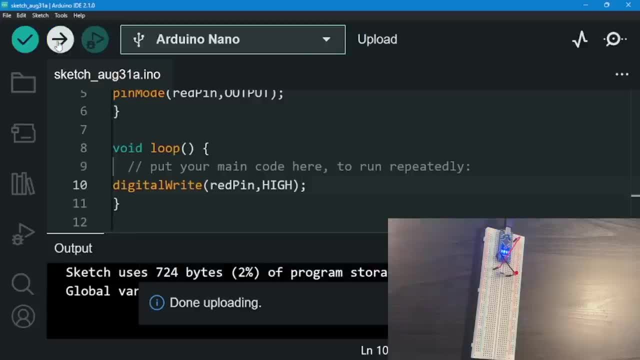 Arduino. let me just upload it right here. it's done compiling, verified the code and done uploading. can you see that it's lighting up? so one thing you need to learn about these digital pins that are marked with a squiggly sign or a dot is we can use them as an analog pin and we can also. 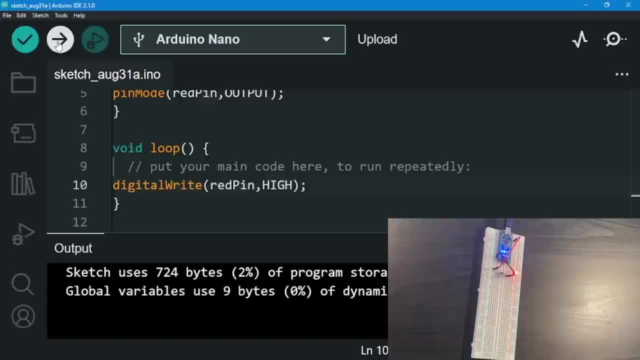 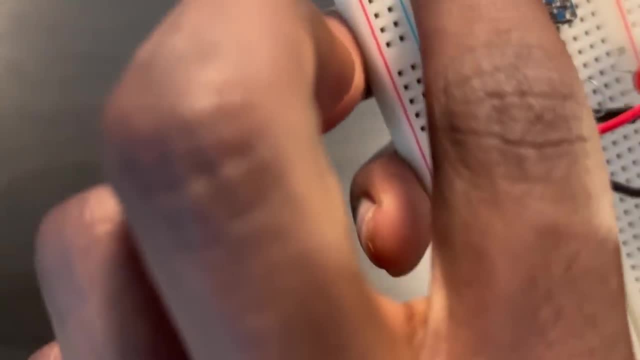 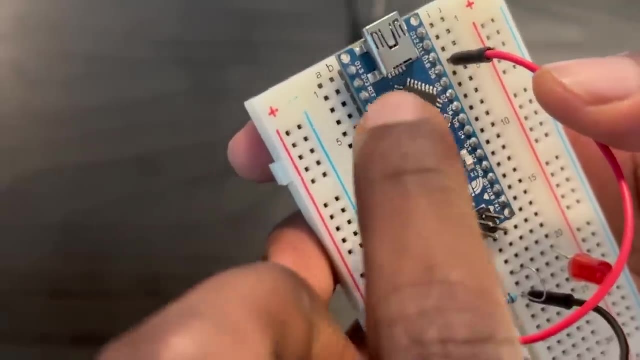 use them as what? as digital pins. I want you guys to keep that in mind, alright? so see you in the next section where we're actually gonna work. we're gonna work with these a pins, with these pins that are exclusively analog pins. you see, these pins, they're exclusively an analog, alright, so they're only analog pins. so 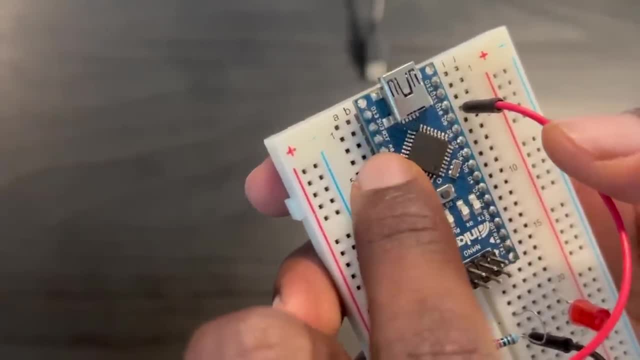 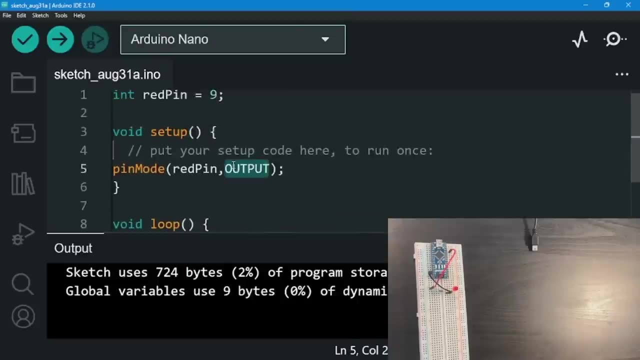 we're gonna actually check them out and for the first time in our lives, we're gonna use pin mode and set it up as an input. so so far they've used pin mode and set it as an input, as you remember here. alright, so we got actually as an 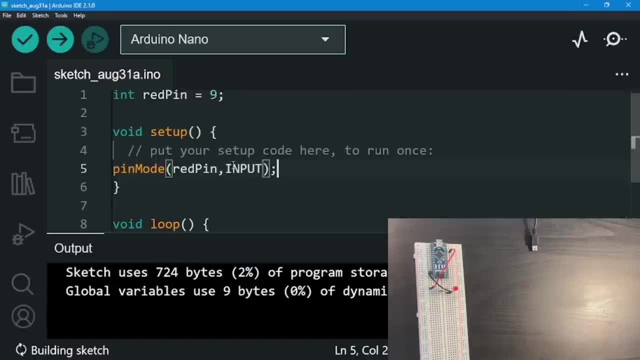 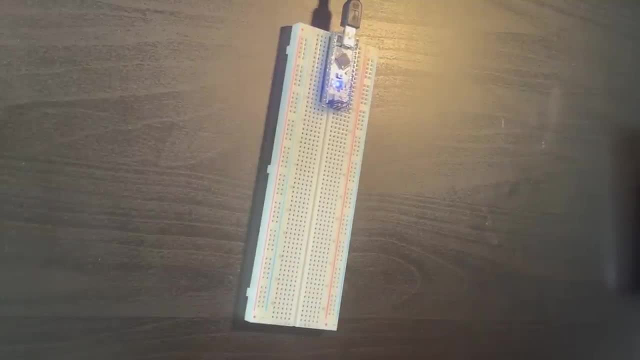 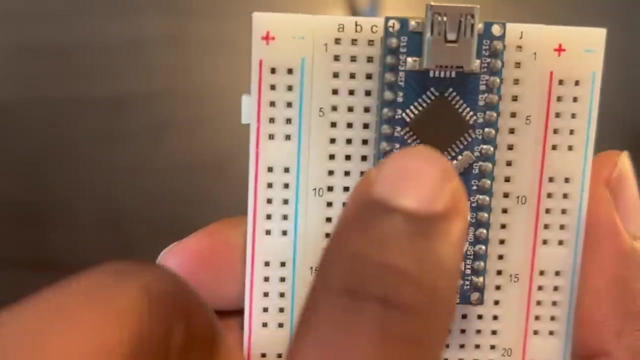 output. so we're gonna set it up right here and use it as an input in the next section. so see you then. right, so let's continue and learn about analog pins. alright, so right here, we've got these pins right here, again marked. let me just unplug my Arduino right here, these pins that are marked with an A and that. 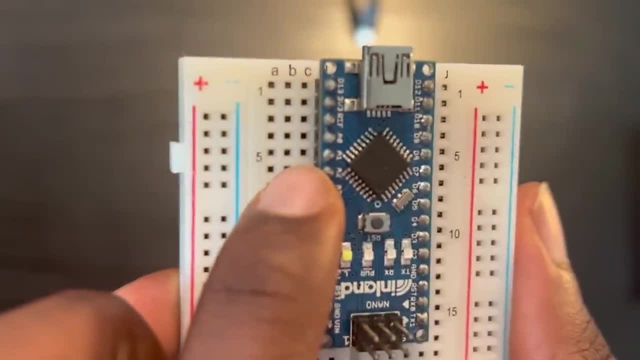 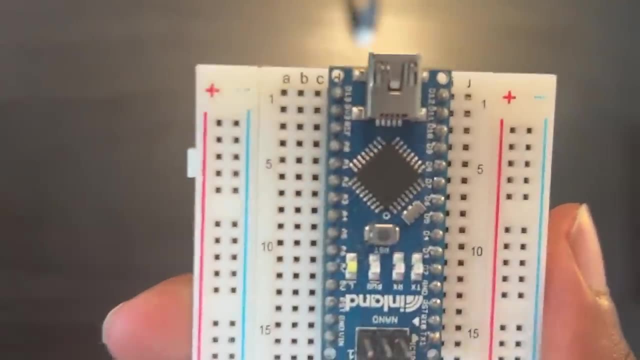 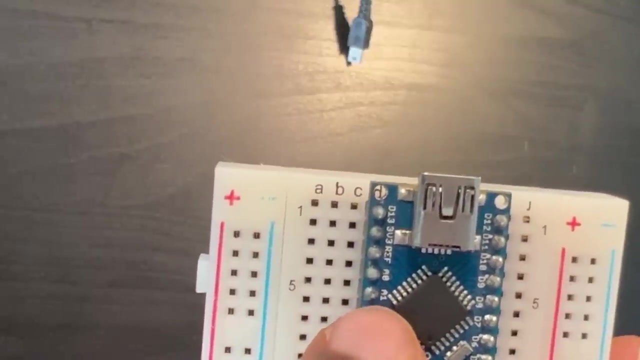 respective number next to them. okay, so the analog pin. so let me again focus here. all right, there we go. it's focusing. let me just go a bit closer, maybe even zoom it better. let's be better. there we go, see those eight pins that are marked with a number and an A. an A and a number next to them. those are: 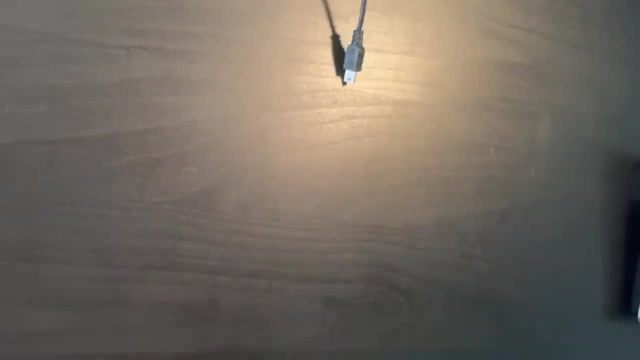 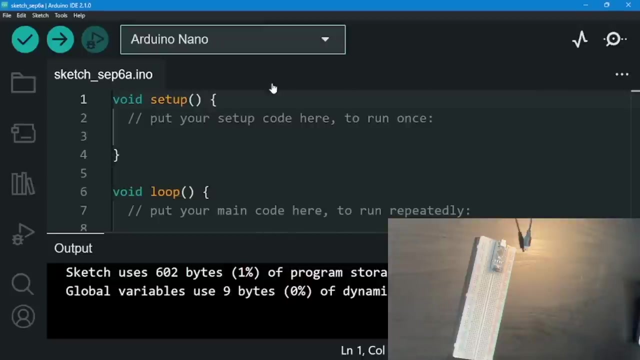 called what? analog pins? okay, I'm just to zoom out for now. all right, so I'm gonna be working them. so let me go over to my screen right here and let me scroll over to my screen and what I'm gonna do here. do this. so let's set up our 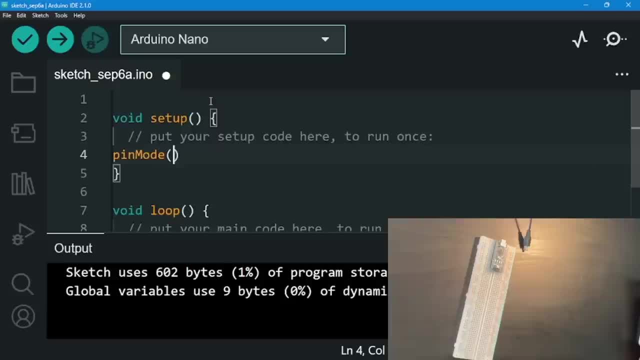 pin. so right here, I'm just gonna say to pin mode again. then I'm gonna choose a random pin. I'm gonna choose a pin E5. okay, it's gonna put this as what? as an input. okay, when we're using these eight pins, we're gonna use them as an input. so 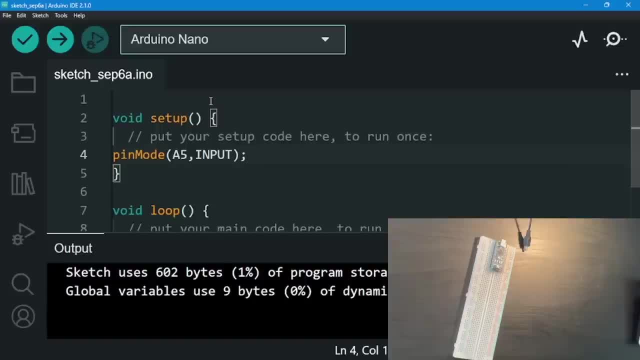 we've worked with digital pins, and we've worked with pins that are analog and also, uh, digital, those ones that are marked with a squiggly sign. I have a dot on there. all right, so far we've used them as a what? as an output, but right. 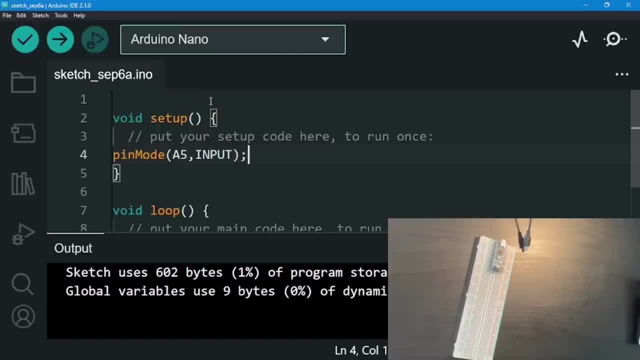 now we're going to use them as what? for the first time, we're going to use them as an input. we're going to use some pins, those pins, as an input. okay, so one thing I did wrong right here is: I do not use a variable again. variables make our life. 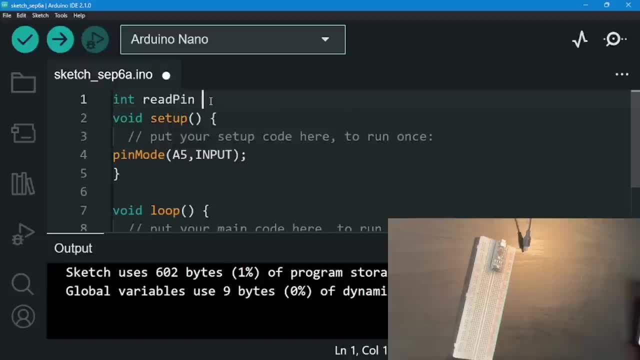 very easy. why not use them? I'm just gonna say: read pin. it will make more sense when I go further to this video. all right, so I'm just gonna say it's read. okay, I'm not gonna use the direct thing, I'm just gonna use a variable. I'm not gonna use direct value of it, okay, so once I'm done, 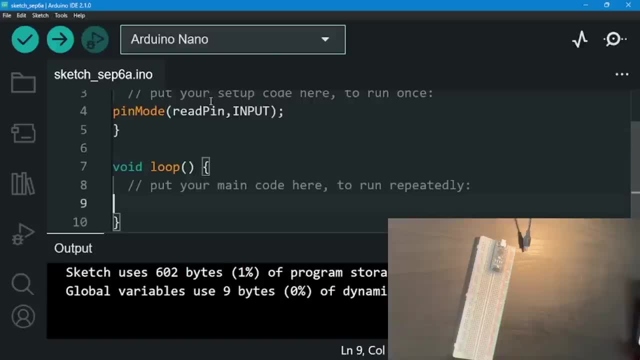 setting it up. what do I need to do? I need to use the analog read command. right, analog? there's something called analog read, as you can see right here. all right, analog read command. so far we've used what analog right? like I'm correct, use analog right. we also use digital right, okay. so for the first time in our lives, 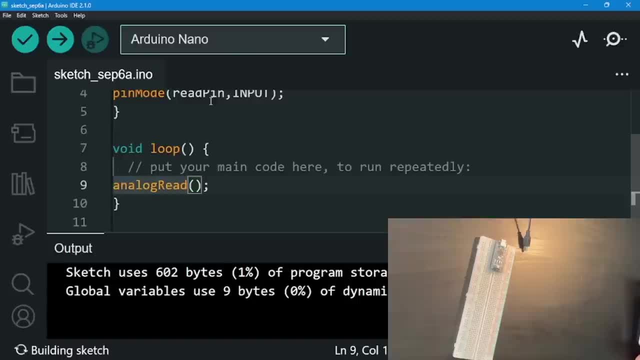 instead of writing, we're going to use what we're going to be using: analog read. okay, to read, okay. so what does analog read do? so, basically, so far, what we've been doing was outputting voltages, if you remember. so, output voltages. right now, what we're going to do is we're going to read voltages. 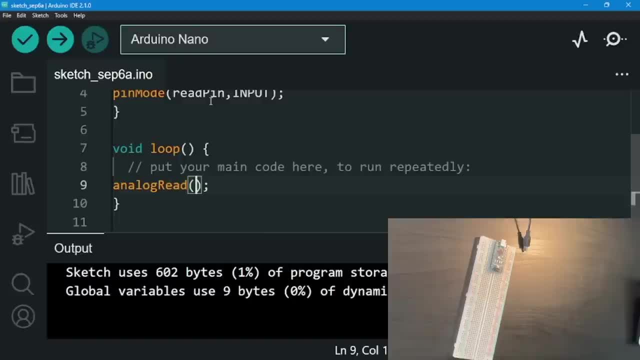 we're going to read voltages, right, okay, so let's just do that right here. so analog read, and what you're going to put right here on the analog read is: is the pin that you're going to be reading with: okay, read pin, okay, all right, that's what. 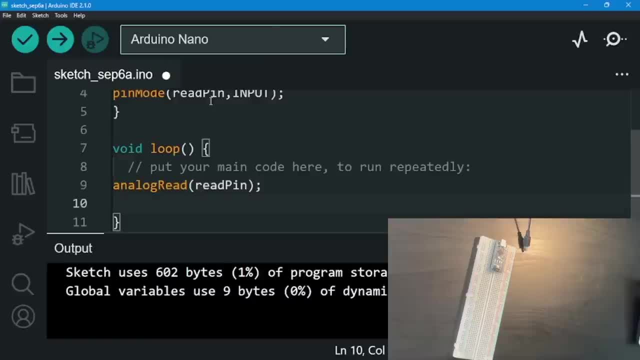 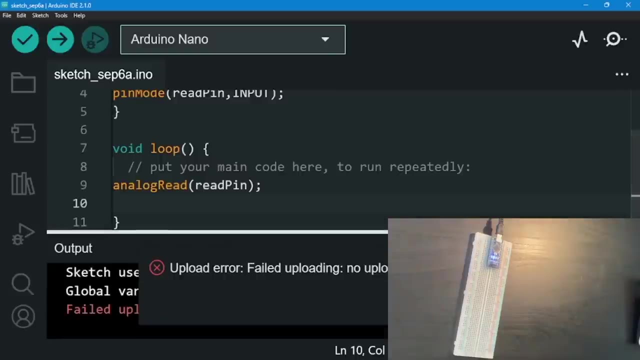 we're going to be using to read a pin. okay, so let me just turn on my Arduino right here, plug it in right here, and then let's upload this code. favor, no upload port provided. all right, let me go to my uh tools and then let me. 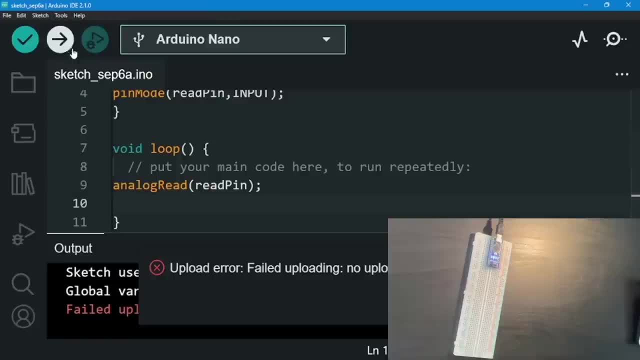 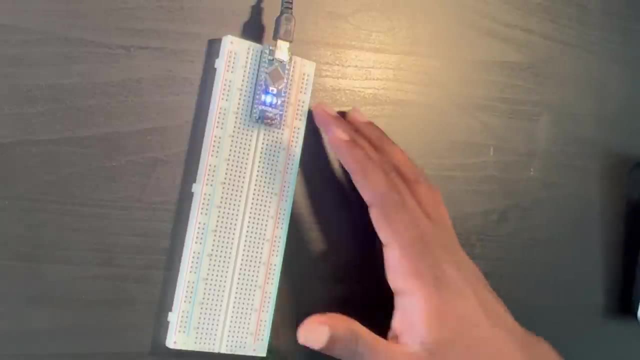 go to my port right here and select the comfort port. now let me upload it. it's done compiling. it's done uploading, so finished uploading. but how am I supposed to see the result? you know, when we were using um output pins, when you're using Apple, what we did. 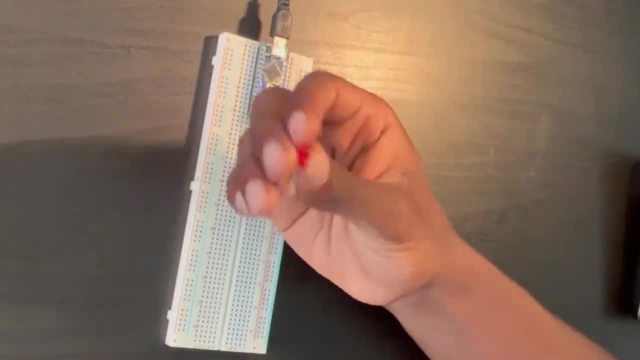 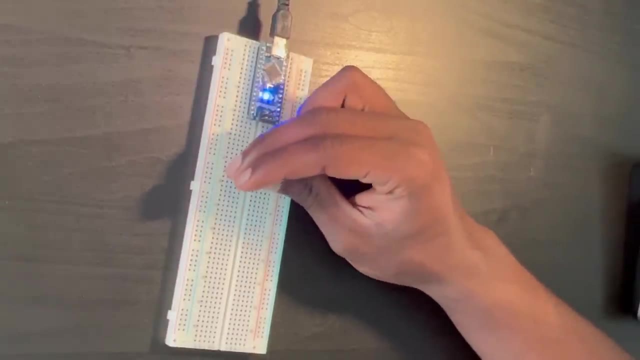 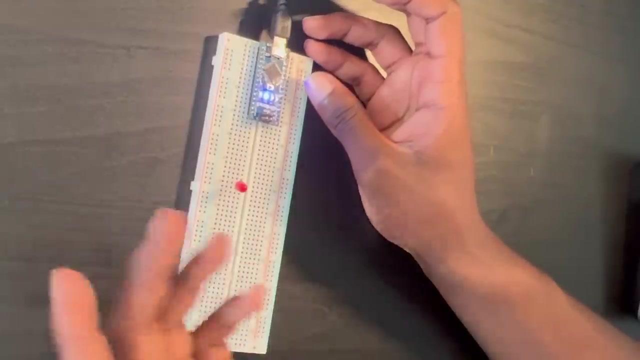 is what we used LED these to see the power and the voltage that they had remember right. so we've been using LEDs to do what? to see? the voltage when they turned on, we said was what? it was five volt. if it was dimmer, we said it was a lower voltage. so we used LEDs to direct us, to basically tell us and to basically 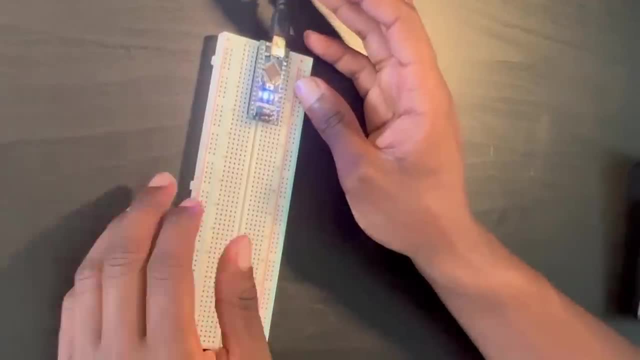 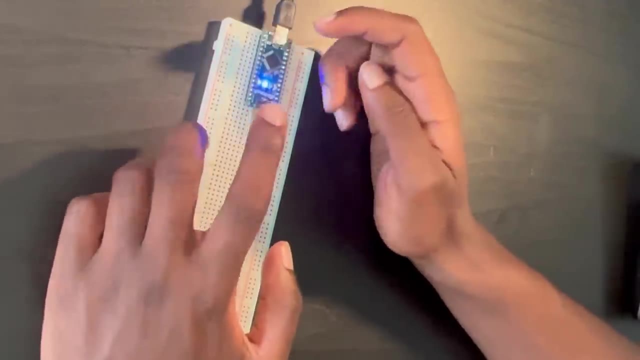 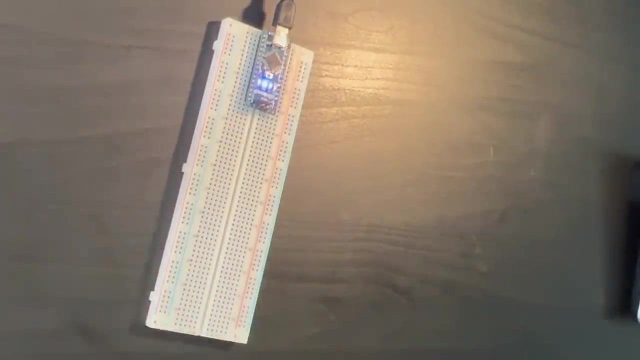 show us that what our- what our pins are outputting, what our pins are outputting, uh, voltage. okay, how do we do it when it's reversed around? so far it was an output, but how do we do it when we're using an input? so, to do that actually, let me just 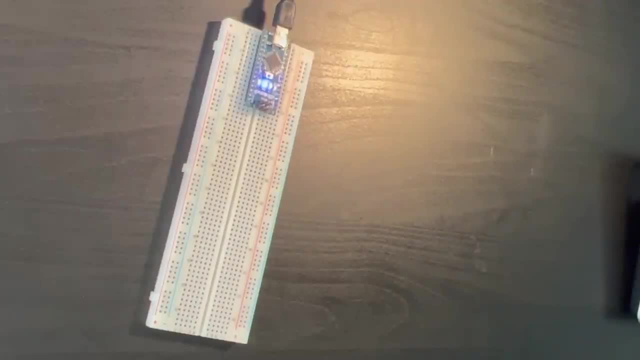 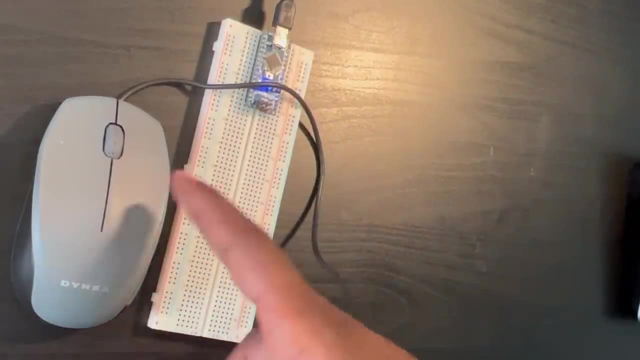 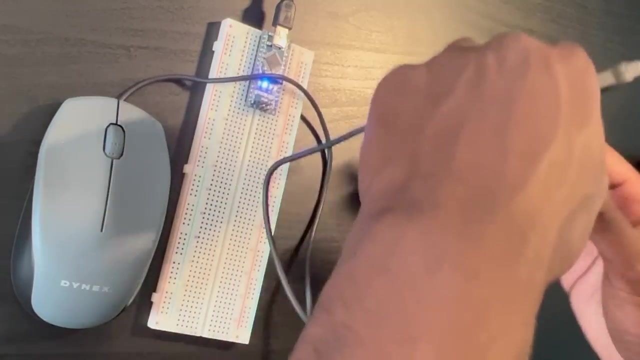 bring the. something that is common- and I think all of you know if you're using computers- is a mouse. okay, so a mouse is a what is it an input device or an output device? it's an input device and basically what we do is we connect it to our computer again. I'm just connected to our computer. 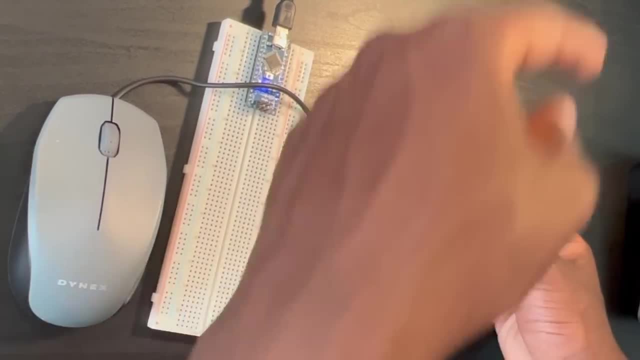 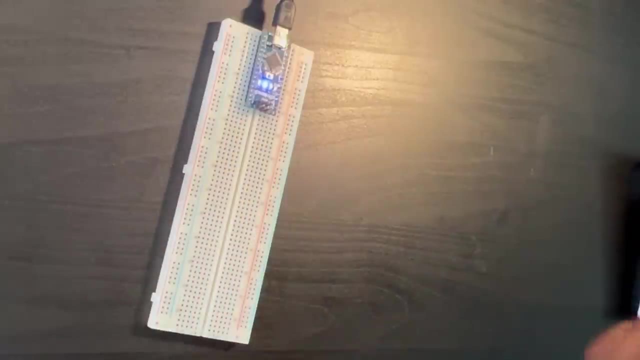 and when we move, we do that, we do what. we see something on our screen. what is that? what is the thing that we see on our screen? it's a pointer. okay, so we see a pointer, so an input device. what do we expect now? we expect is what to see? the 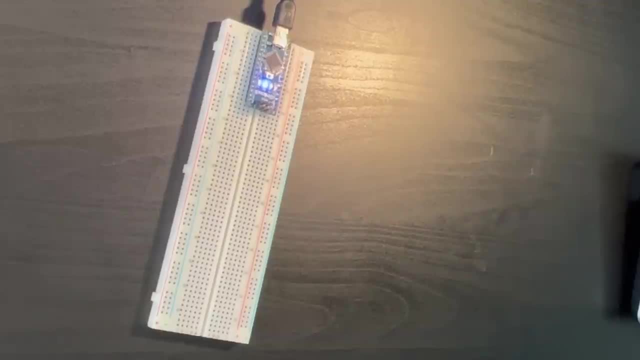 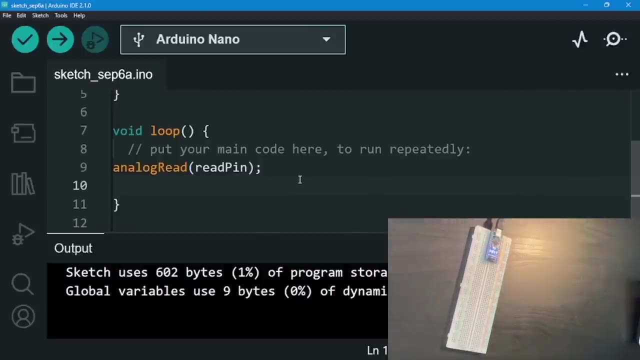 results to happen on the screen. that's what we expect. okay, so to do that and to actually see something on our screen, we're going to use something called serial monitors. okay, so, we're going to use something called what serial monitors. so we're going to do a serial dot begin. okay. 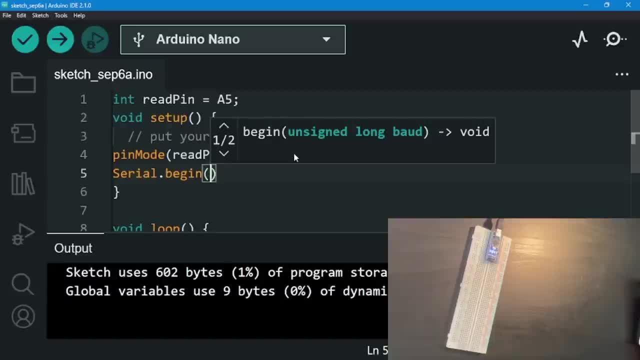 so you might be wondering: what is a baud rate? a baud rate is a: the speed at which. it's basically the speed at which information is transferred. okay, I want you to think of it like that: don't go further or don't go deeper, as it mostly does not matter, but to catch it just for. 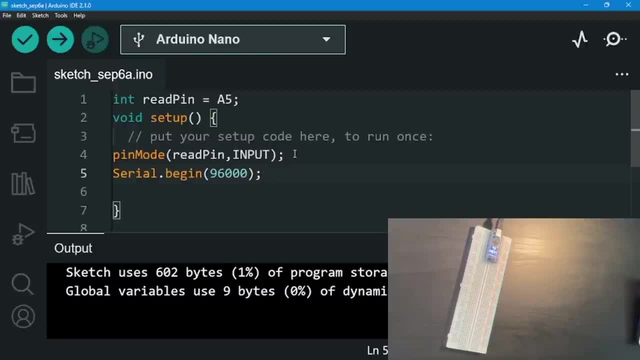 the sake of knowing and for the sake of knowledge. to catch it is: it's what? it's just the speed at which, what? the speed at which information is transferred from your computer to other devices. okay, that's just the thing you should be thinking of. bottom it says okay. 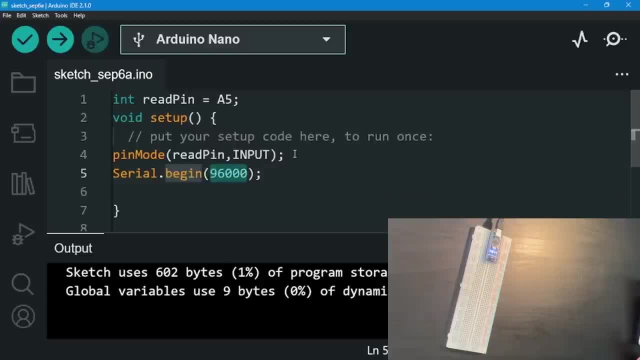 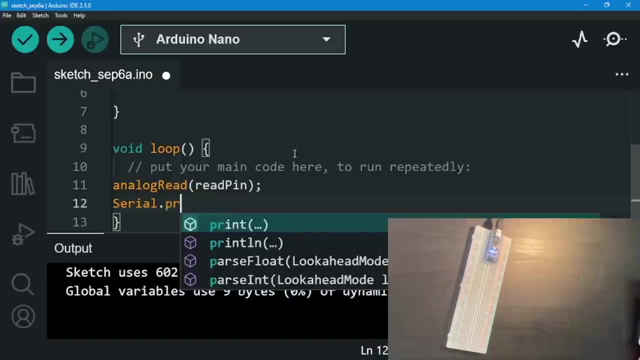 serial dot begin: 96 000.. I set it as 96 000 as it's the most popular baud rate. all right, it's the most popular one. okay, so I just started my serial monitor right here and what I need to do is quite simple, I need to say, is serial dot print. so I wanted to print something, for example, let's: 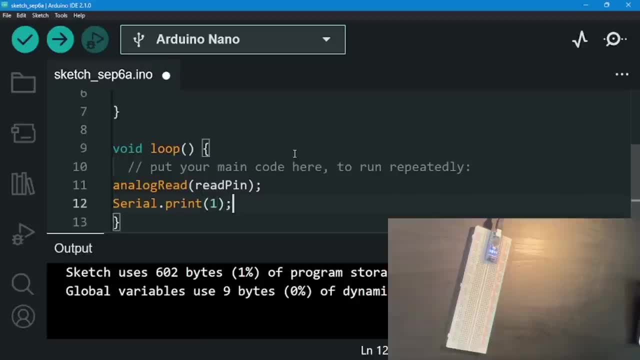 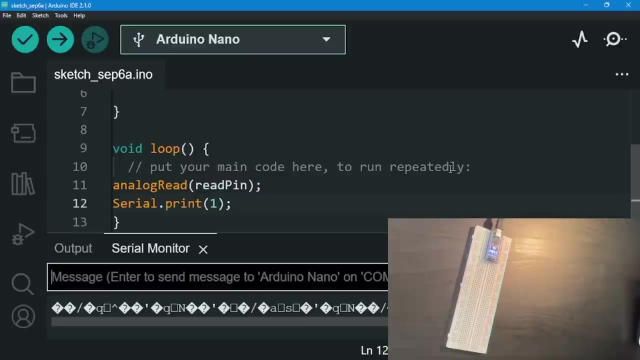 say I wanted to print the number one. okay, just say we want to print the number one, number one for now, so let me upload it right here. okay, all right, it's done compiling, it's done uploading, and you go to your tab right here where it says serial monitor. I'm gonna touch that, okay. 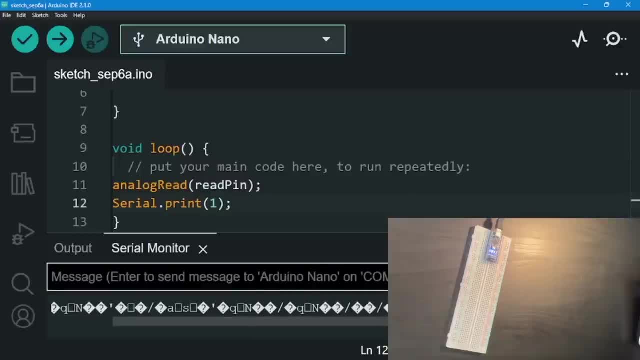 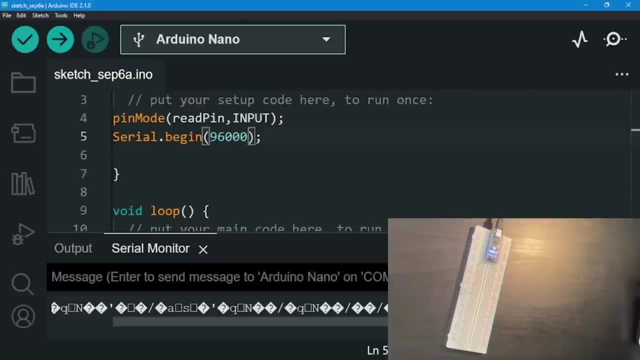 can you see what's going on? I said 96 000 baud, as you can see, it automatically set it up. because what? and there's something wrong right here. what did I do? I said it says 9600 baud right here and I used it. I'm supposed to say 9600, so let me upload it again. you see that I'm getting an error message. 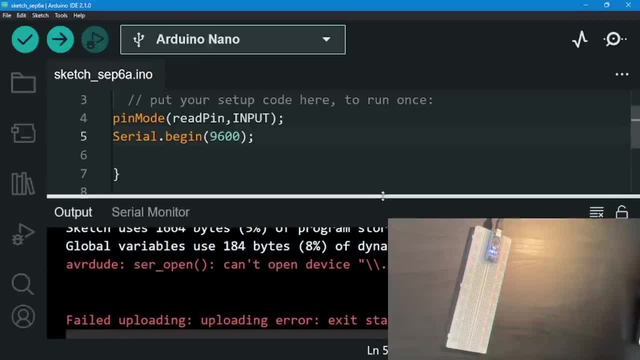 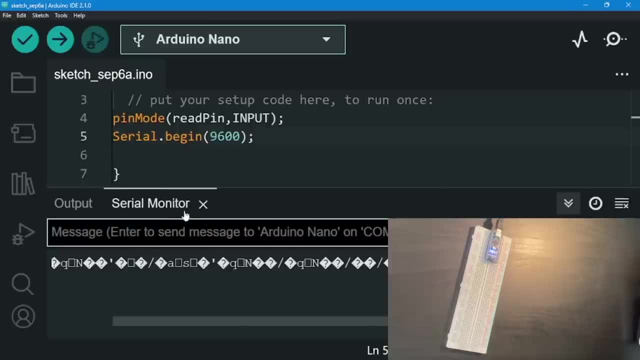 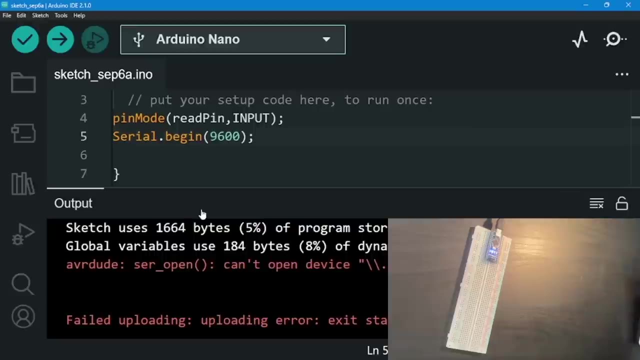 right here. so for those of you who don't know is you can't run your, you can't upload or verify your sketch without removing the serial monitor, so you always have to turn it off before, uh, uploading or moving, all right, verifying your code. so I have to always turn it off and I do that, and let me just 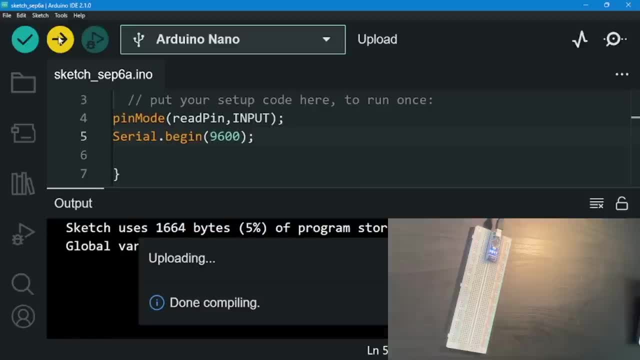 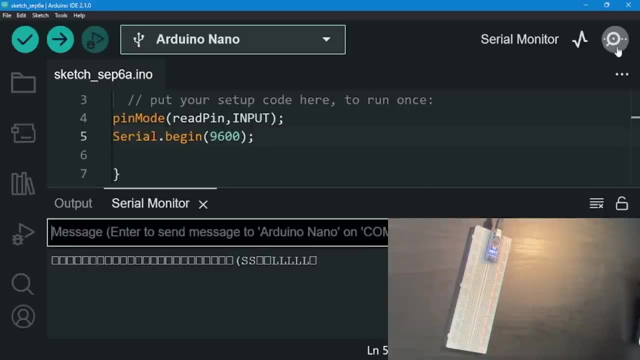 upload it right here. there we go. it's done compiling, it's done uploading, so always turn off your serial monitor. uh, when you're uploading your code, let me just upload it right here. can you see it? it's uploading one at very fast speed. look at it. one, one, one, one one, you can. 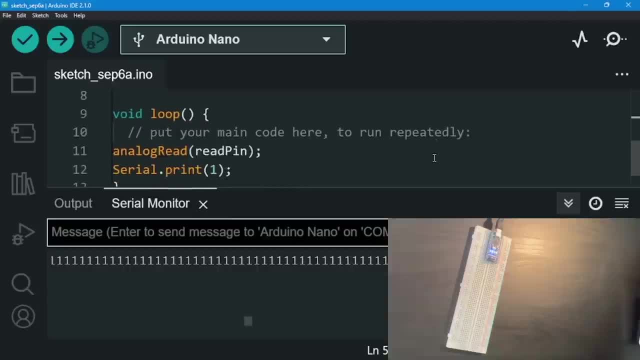 see how fast it is. look at how the pointer is moving. it's very fast. okay, so I just said it's print one. that's all I'm gonna do. it's basically like the print function that we use on uh, on uh, Python. okay, alright, so I wanted to print the value of this. I wanted to print the. 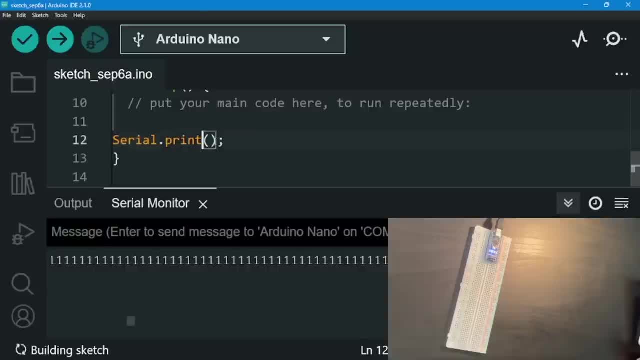 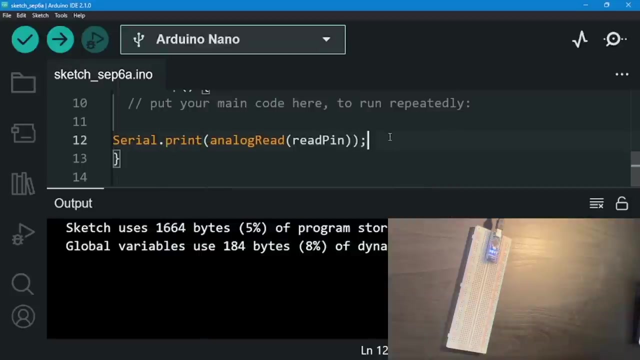 value of this. okay, I just wanted to print the value of this. let me just do that. set it up, just turn off the semicolon right here. first things first. what should I do? I should what? turn off the serial monitor, okay, just turn it off. and you know what? it's going too fast for me. I'm just gonna give it a delay. so 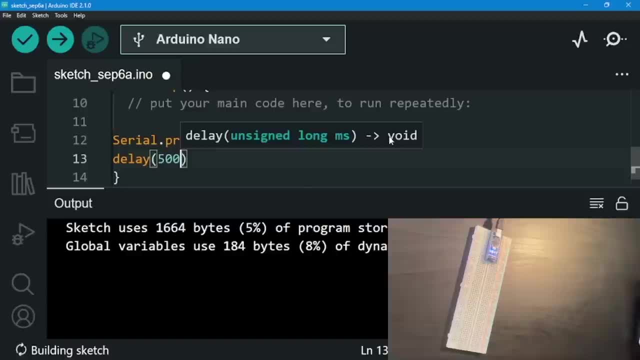 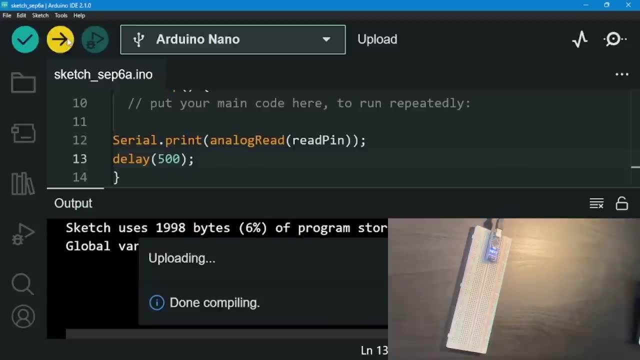 I want it to delay for what? let it delay for maybe a 500 milliseconds, okay, so basically half a second. I just wanted to delay for half a second because it's going too fast for me. okay, it's done compiling and it's done uploading, so let 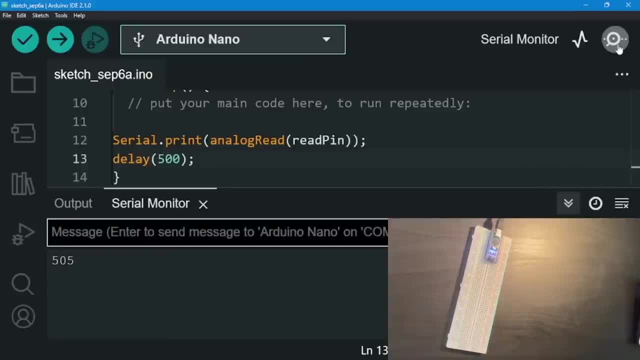 me go back to my serial monitor right here and we're receiving. that's very confusing, isn't? I mean, is it? is this one 50? because it printed it out. it's very fast speed. so this is 50. then this is a 50 here, or is it 505? or is this 500, 5054, are they? 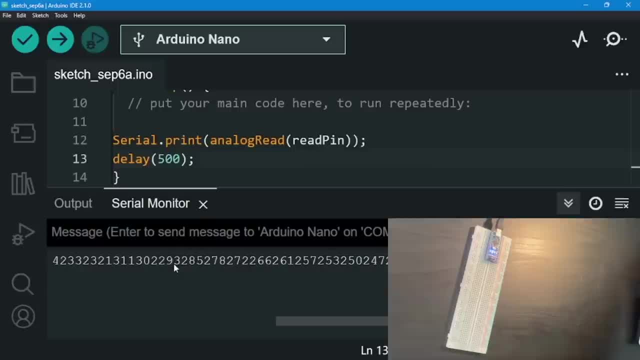 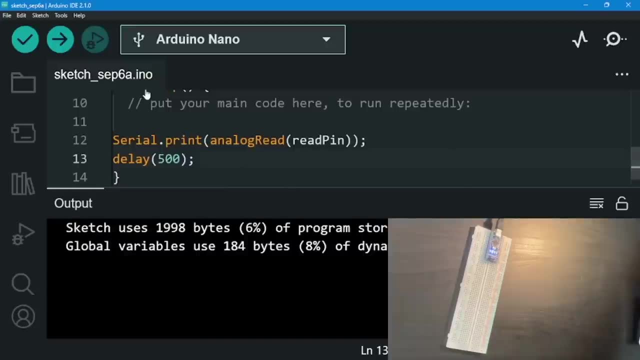 together or what. I can't see it until it uploads it right here. okay, this is very hard to keep up, so what I'm gonna do here is turn off the serial monitor right here. okay, I'm just gonna do that. and what I'm gonna do right here to say 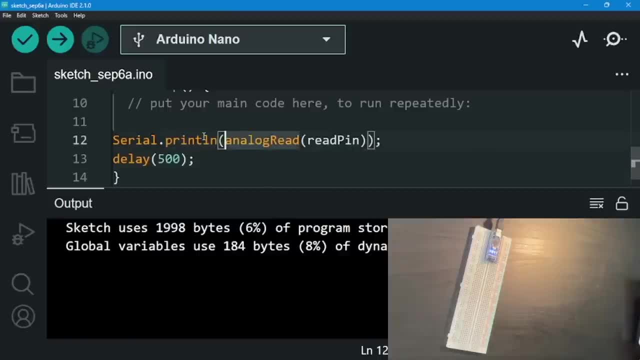 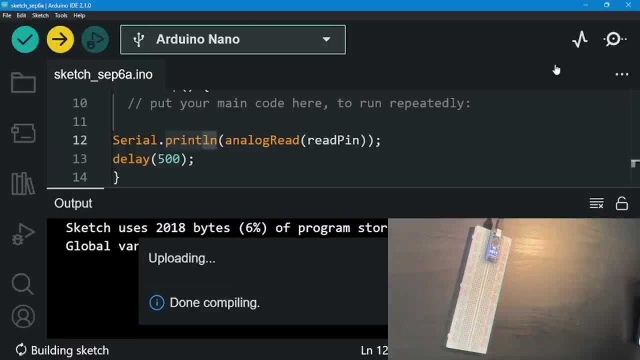 print and add a link at the very end. what this does is basically it prints out everything at a new line. okay, so print that out at a new line. every print is going to have its own what its own single line, all right. so with that in mind, let me just upload it right here and let's see what happens to the serial monitor. 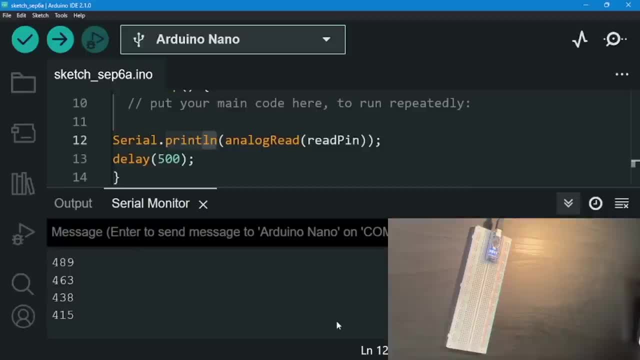 come forth here. all right, there you go. it's working actually. all right, you see it. it's just fluctuating, saying 321, receiving 280, 273, 256, 255, okay, okay, okay, this number does not make mostly sense, does it? i don't think it does, so what i'm gonna do is all right. what i'm gonna do is this: 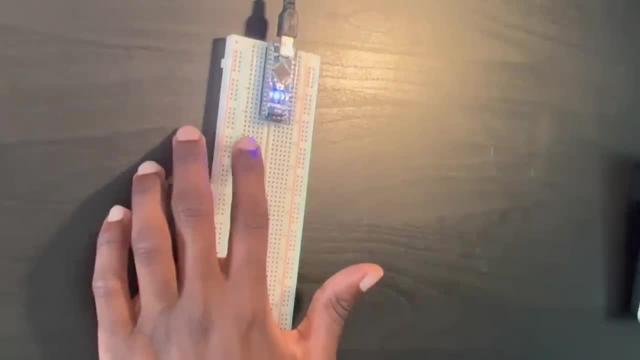 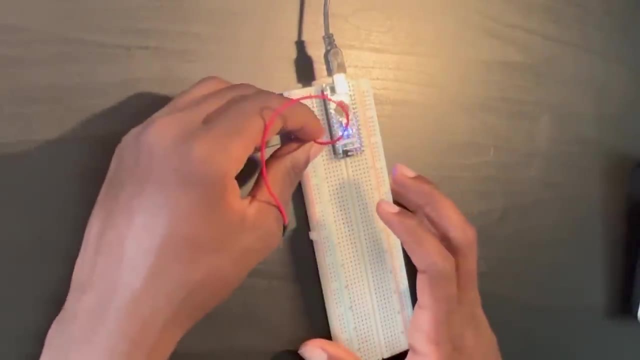 so let me just try to do as well. i'm just gonna read off of the five volt voltage, all right, so what i'm gonna do here is: i have an analog pin right here. okay, i have this analog pin again. what analog pin am i using for this? i'm gonna be using analog pin five. let me just bring analog pin five. 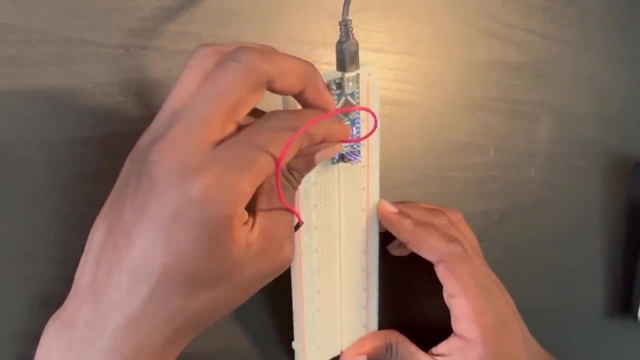 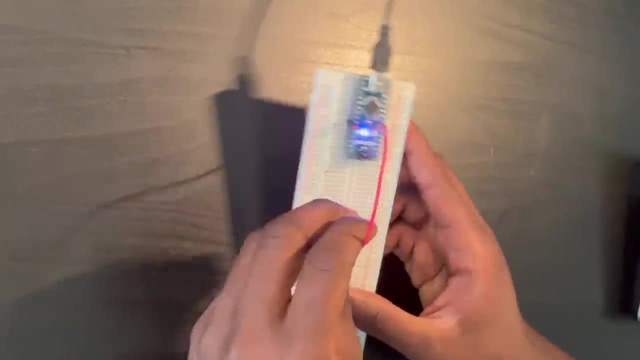 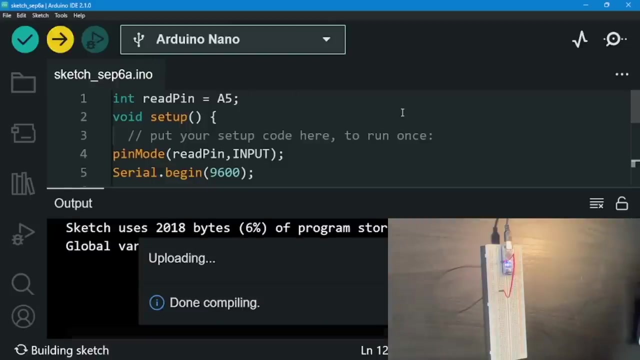 right here. i'm just connecting it right here. okay. analog pin five. let me just make sure that i actually connect that analog pin five and that i'm not connected to any other pin. analog pin five. okay, let me just connect it here. okay, so let's just again upload this code. it's already uploaded. i just 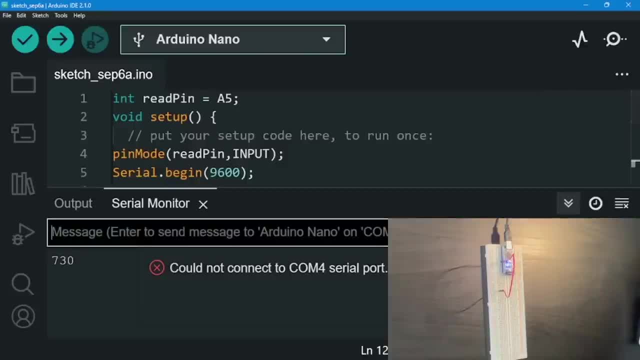 i just uploaded it again so that it restarts, all right. then receive again these weird numbers, because i still don't know what are these, okay, what they are? i still don't know that. so i'm receiving 10, 23, 9, 86, all right, so we have to make something of this. 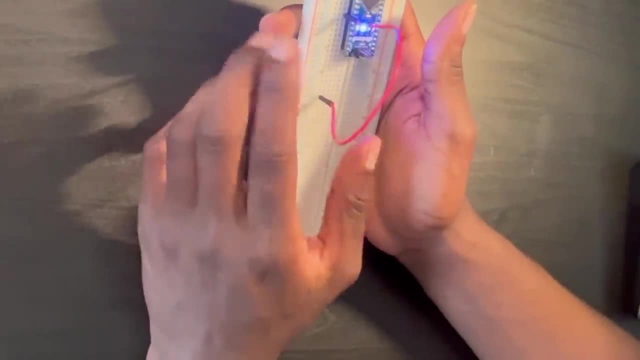 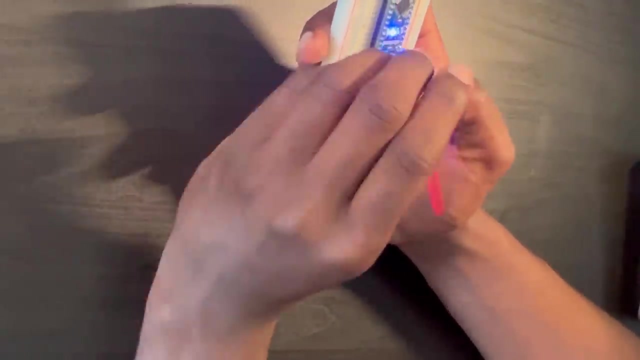 numbers, okay. so what i'm gonna do right here, okay, is you know what? this is supposed to read? the voltage. again, as i told you guys, it's supposed to read the voltage that is coming from what? from our arduino. so let me go right here. i have my a6 pin right here. can you see it? i have an a6 pin. 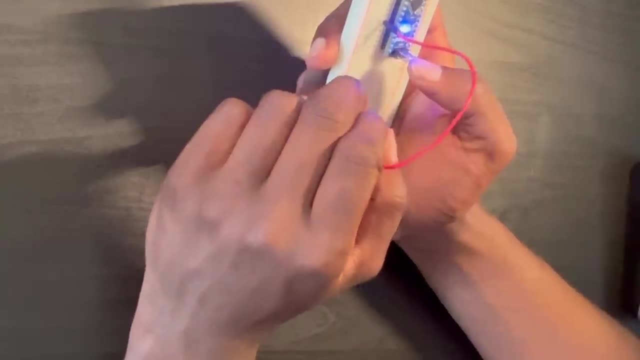 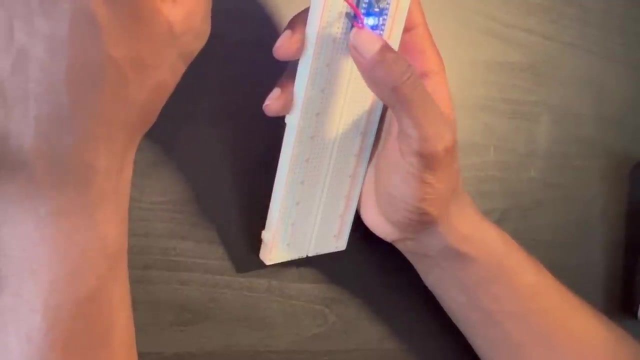 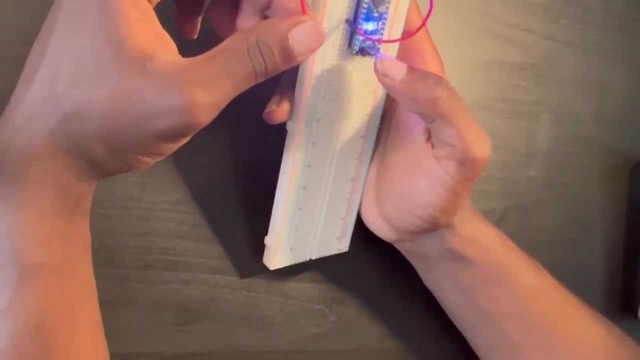 i have the five volt pin right here. but i am very, very intent. i am very, very confused. should i connect this together or should i not? i am really hesitant about the circuit. should i connect a6 with the five volt? because if i do, am i short the circuit. if i short the circuit, basically. 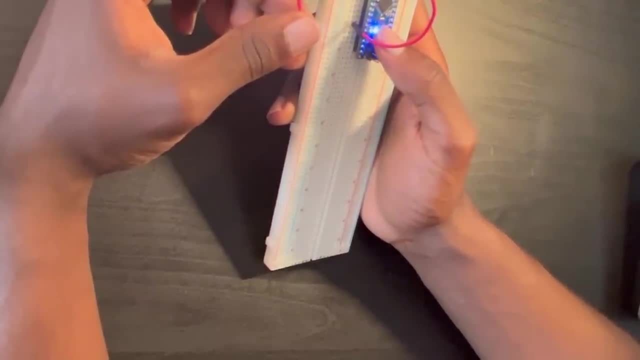 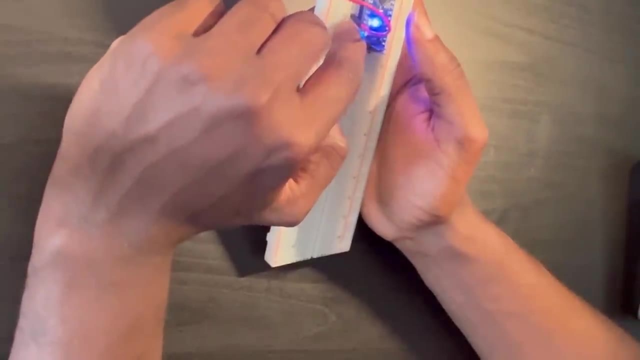 i might fry my arduino, you know. so i'm a bit hesitant on connecting them directly to connecting my pin right here with a five volt, because i'm not used to doing that. we're used to what? connecting five volt and then going through resistance and then going to what? to the gnd. all right if i'm. 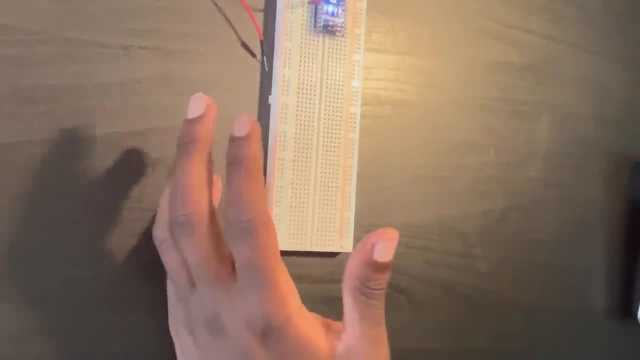 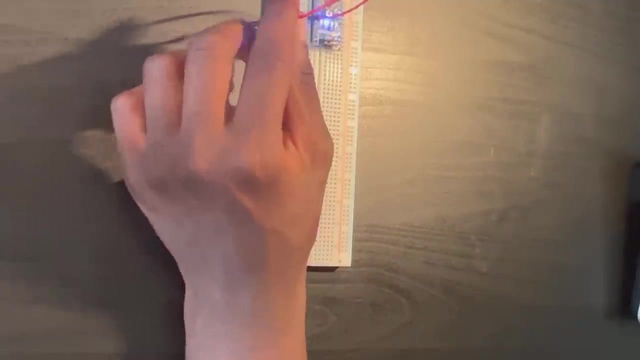 correct. so how do i do that then? how do i do that? how do i check? um, you know i'm very hesitant about this uh circuit right here. i don't want to connect the a5 pin directly to the five volt pin because i might short the circuit, but i want to. 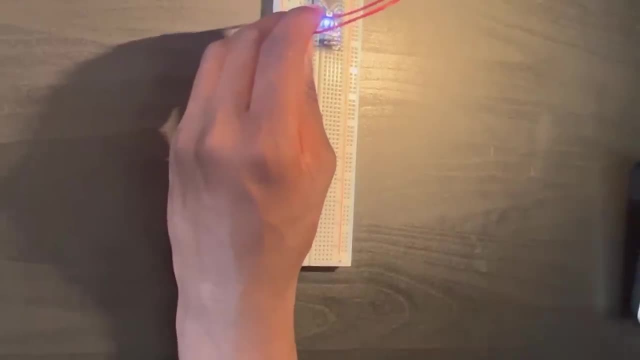 do it so that you know. the answer it gives me is five volt. i want to check it. so i'm a bit hesitant on this, on this uh circuit. so rather than just you know doing this and hoping for the best, it's better to do what again? it's better to run a simulator. so i'm just going to go to my screen. 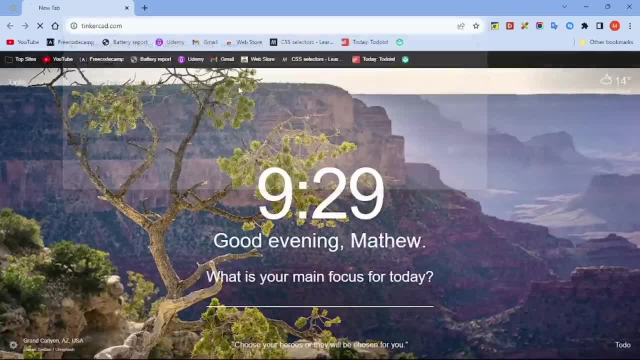 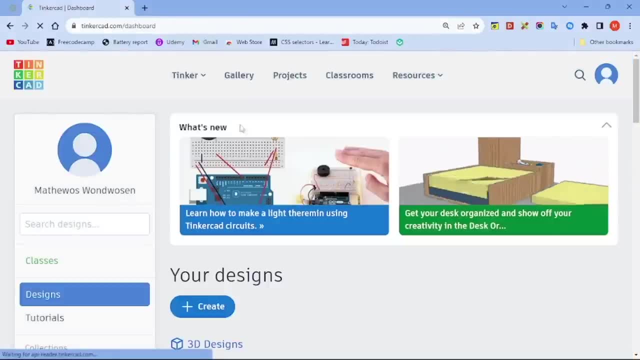 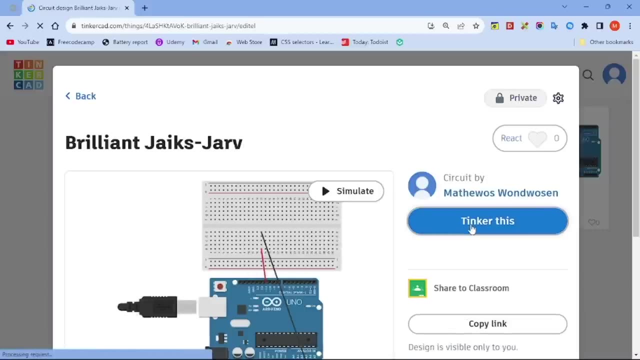 right here, turn on chrome, go to simulator. right here you. okay, that's what i'm gonna do. i mean, that makes my life a bit easier, okay, so again, let me just go right here and i have it right here. all right, let me just open this so i can simulate it. all right. 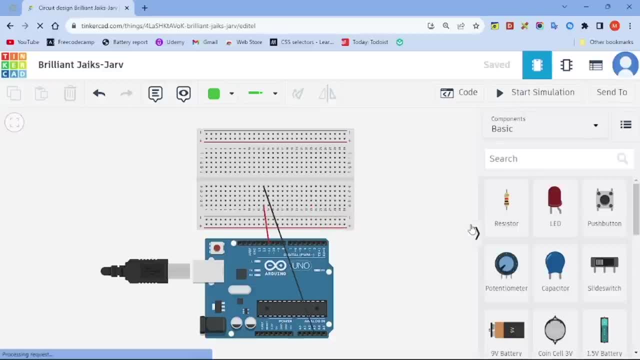 let's just check you know what happens here. does something bad happen? okay, so i have, uh, my analog pin here connected with the digital pin. i'm going to change that to a five volt pin. let's see what happens with the final pin. my five volt pin is right here. 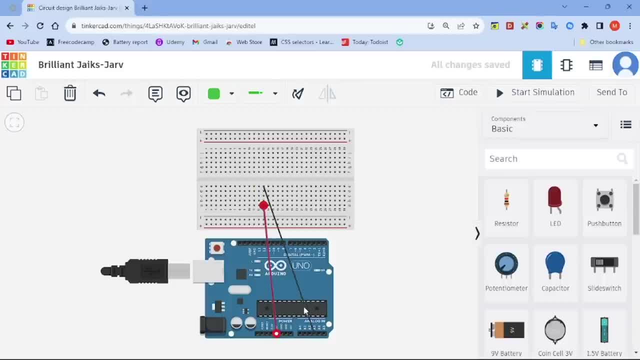 there's only five little pin? okay, and i have wait. what my analog bean? okay, i have an analog pin. however, instead of connecting it like this, it's better. how about i just connect them directly? you know, let me just turn both off, and i'm gonna do this. five volt pin. 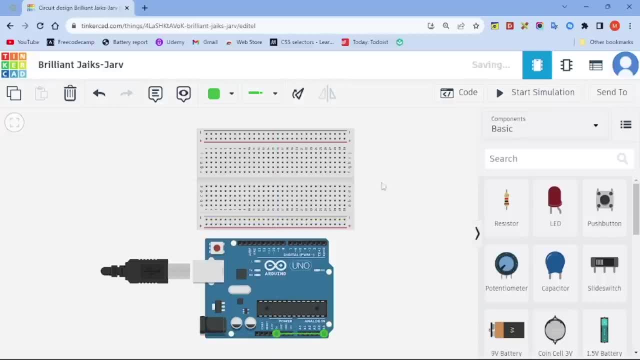 connect directly. let's think to one of the analog pins. this keys a5. let me just start the simulation here. let's see what happens: 3, 1, 1, 10, 20, 13, 40, 21, 21 happened. so far nothing happened. everything seems fine, doesn't it? so far seems fine, nothing is going. 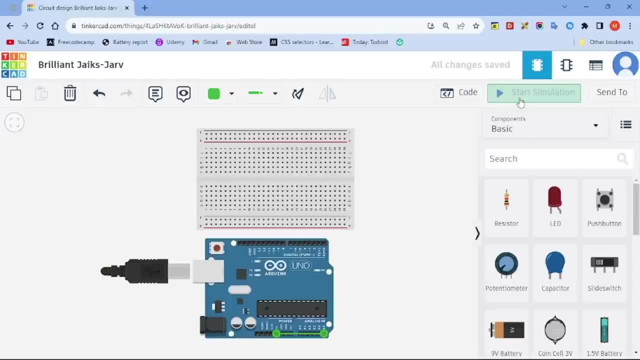 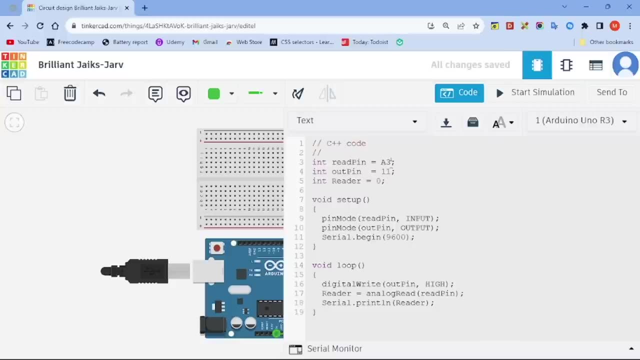 on. i mean, let me just check my code right. here is my code. good, better write down. and just did i set a5 to read. i said a3 as a root pin. i just want a5 to be a read pin. i don't need this because i'm 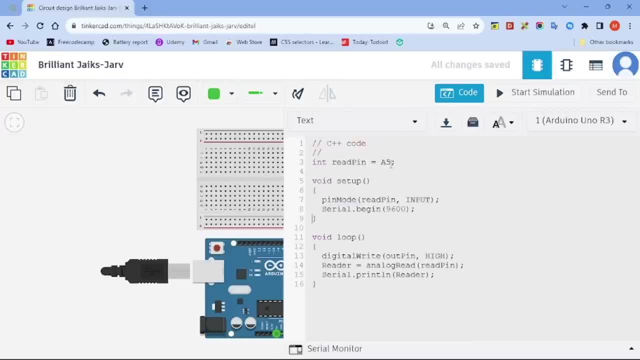 using the firebolt again. i don't need this. i just needed my serial. you know serial topic in 9600. i already set that up. all i need to do is what um say analog. i said reader, a variable reader, right here. i set it to a lot we've been, i don't need that right now. let me just copy this. let me. 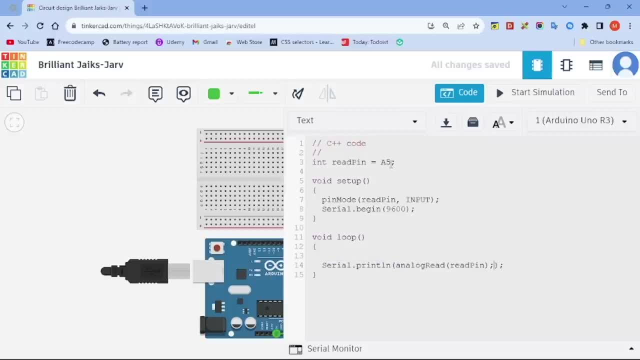 just go back, let's just write it down as if the one that i already wrote down on the uh, on the arduino. okay, so that's what i'm gonna do. so, yeah, i think that's my code for now. let's start my simulation right here. 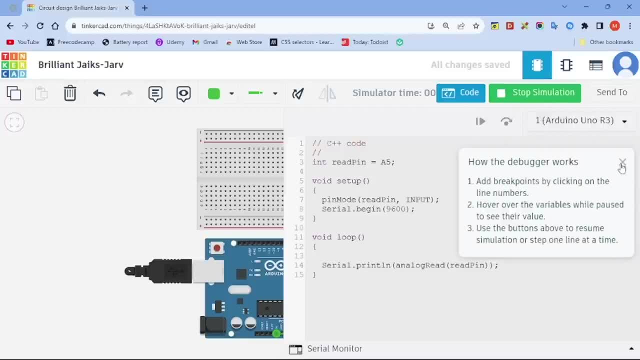 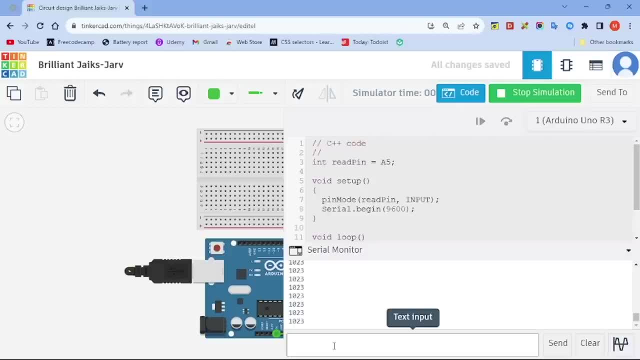 my simulator told me that it's fine to connect an arduino a pin with a. what with a five volt pin? did not say it's correct. you know to put it together, but like, let's see what happens if i connect an a pin while we're here, let's just 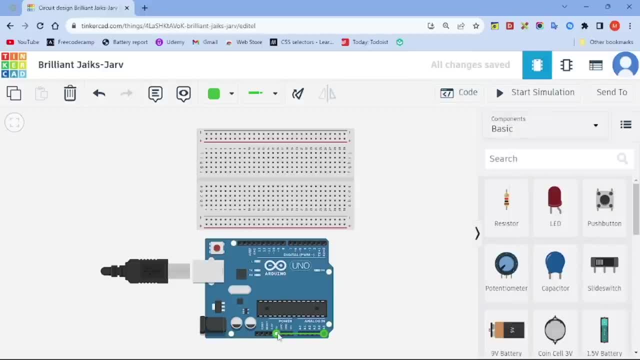 check what happens if i connect: uh, maybe an additional pin. all right, there's still pin, maybe eight. you see, there's still pin eight to um to a five-volt pin. right here let's just say i want to connect to a five-volt, but what happens? you know what will possibly happen um. 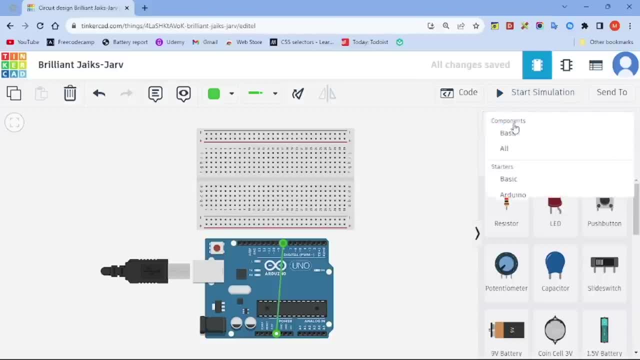 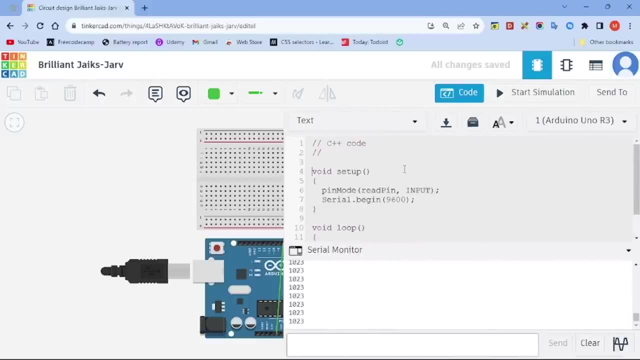 let me just start similarly simulation right here. maybe let me start that. before doing that, though, let me go on my code and let's just let's just write it to become high. all right, let me just do that. okay, i received 10, 23 again. um, i'm gonna get back to that, okay, but i just want to check. 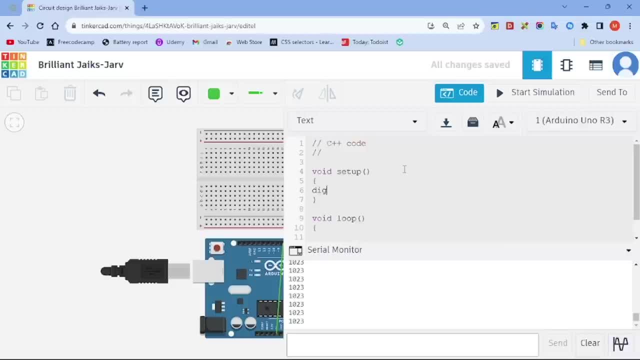 again, what's going to happen when i connect the digital pin with uh, with a five volt pin. so i'm just going to pin node and what i need to do, set up the digital pin eight, eight and say what does an output? i want to use it as an output. 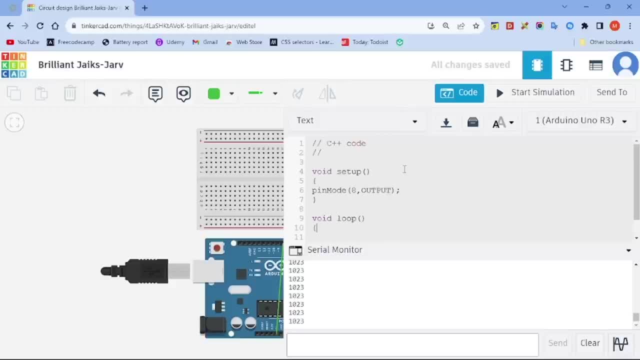 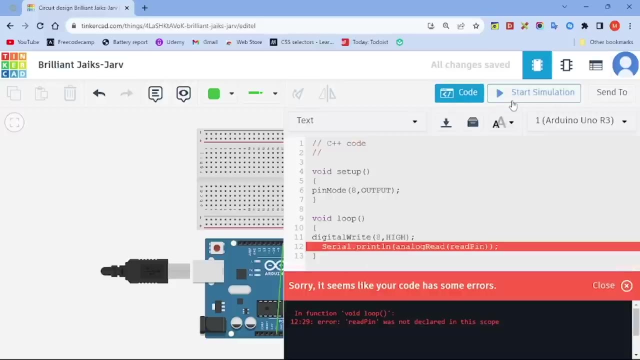 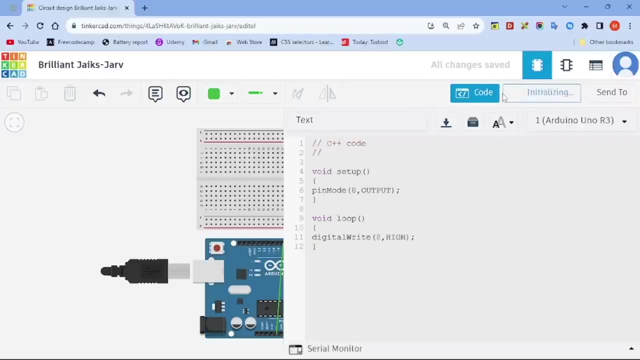 what else do i want to do? one final thing i want to do is what i want to what i want it to be. so i'm just going to say is what eight said that to what? let's see what happens when you start simulation. what happened, saying, okay, this one has an error right here. okay, let me start right now. 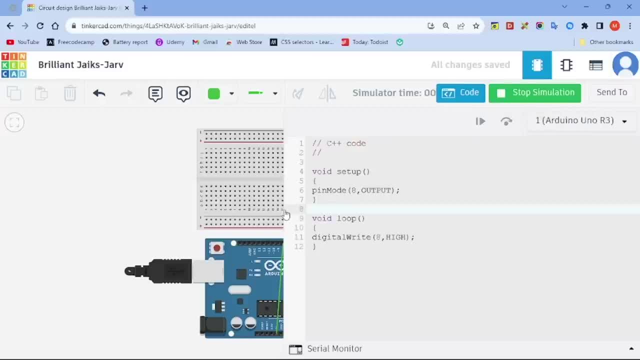 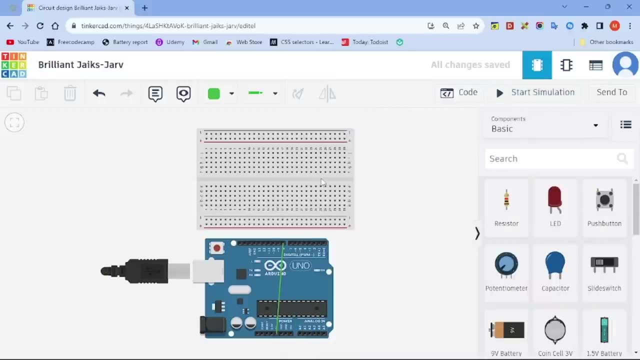 seems fine. yeah, it seems fine. there's no error coming from my uh simulator telling me you should not do this or something. it seems fine because it does not make a full circuit. but one thing that's not fine. that's definitely not fine, for example, is connecting the five volt pin with the gn deep. and let me 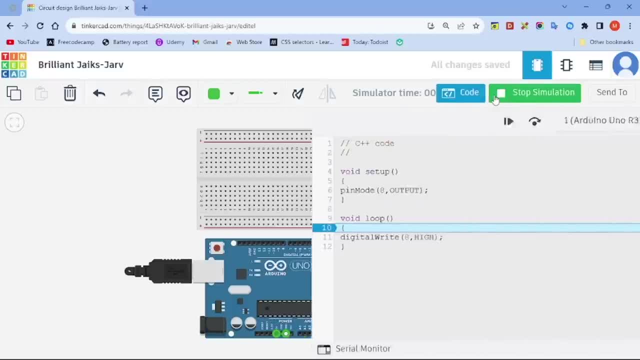 just connect it directly five volt in the gnd. let me just start this simulation. if i do that, i might tell you right here. but what happens is basically what it's basically frying your argument me, what it does not tell me if it's fine or not. okay, it just does not tell me that it's not. 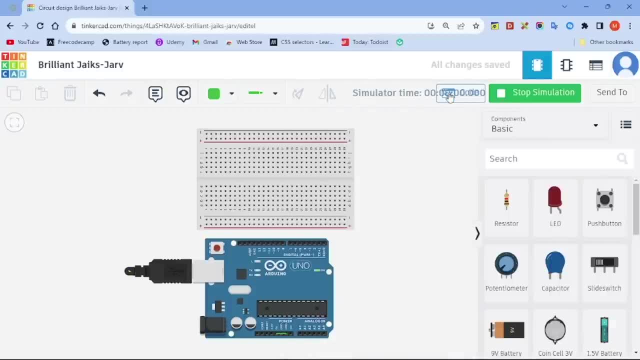 warning me about connecting it directly with the five volt, the gnd, because it's very dangerous to do that, because, again, what i said is shorting is going to happen and basically what's going to happen? it's basically going to fry hard meal. so you see that it's fine. but if i go to another, 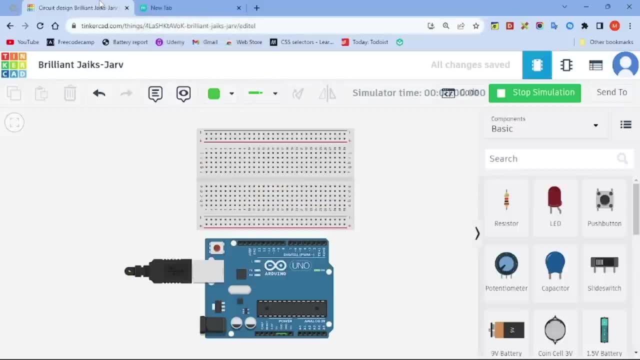 maybe simulator. if you search for another simulator right here, it's going to say it's not right anyways. so, um, let's go back to actually uh what it was. so let me just go back to control z and let me just stop the simulation and let me just uh get that 10 to anything right here. the. 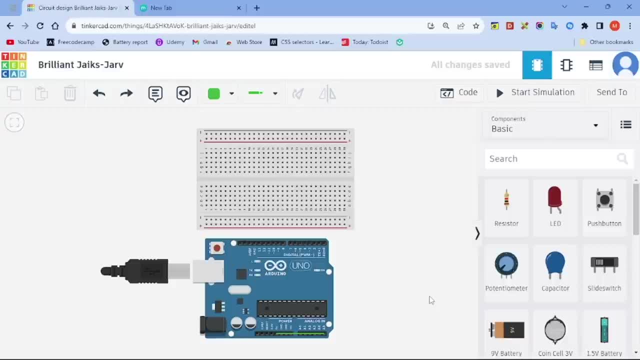 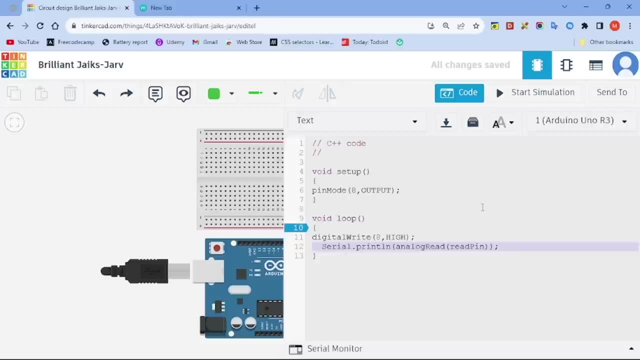 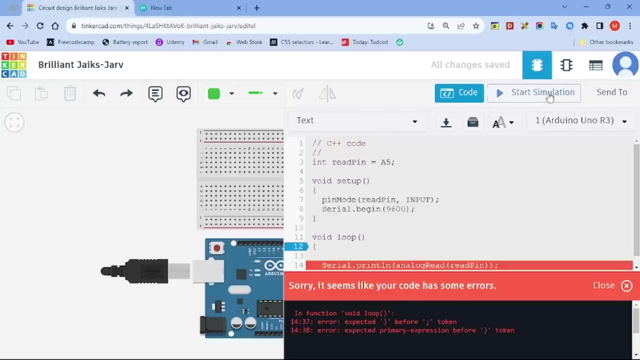 number 10 to anything. okay, let me just go back here. okay, we connect this directly. there. we go back to my code. let me just okay, okay, so let's start the simulation again. what did that do right here? i put a semicolon before this, all right, so let me start right now. 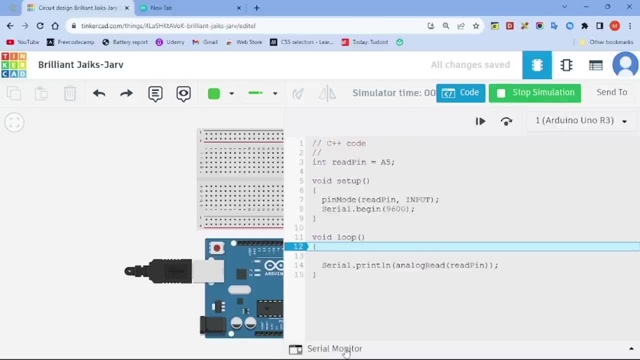 okay, seems fine. let me go to my serial monitor. okay, it says 10 23, 10 23, 10, 23. so i want to explain what this number is. it's like the number that we used at zero and 255 on the animal number. so i'm going to go to my serial monitor and i'm going to go to my serial monitor. 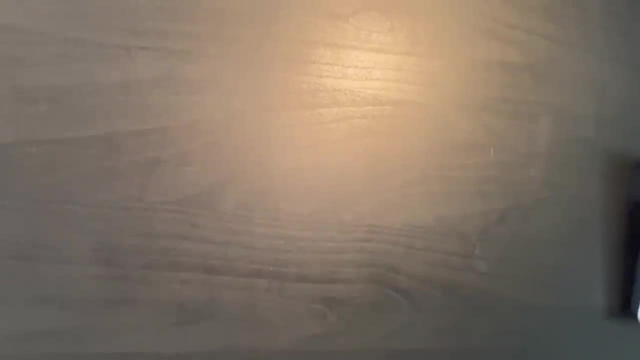 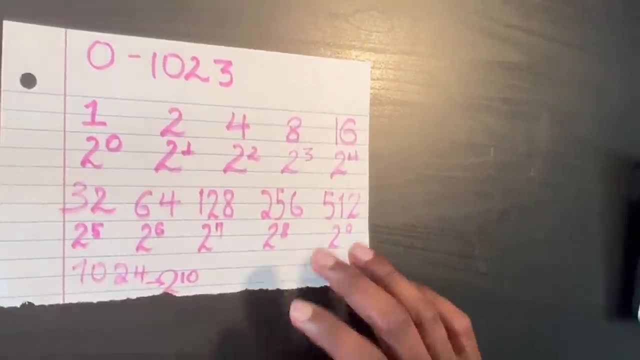 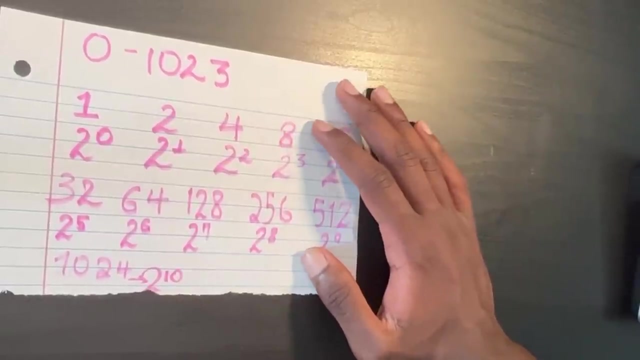 right command, we're using 255. so let me just explain this right here. let me just bring the paper and explain this right here. okay, so the same thing we did on uh, we basically did on the uh 255 to zero value when we were talking about uh, the analog right command. okay, so, look, we have one. 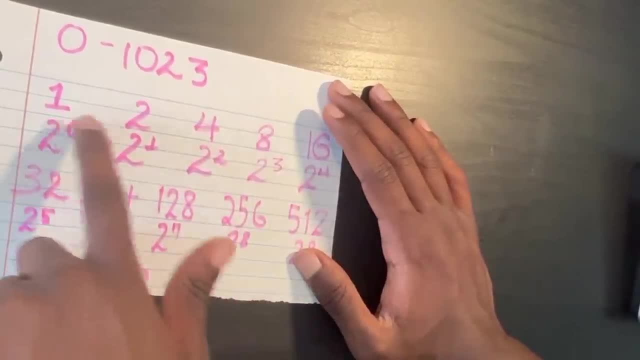 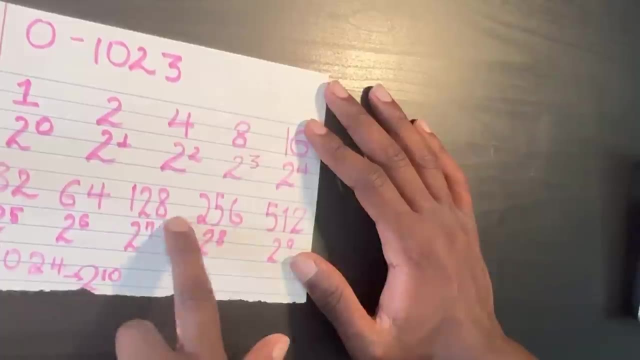 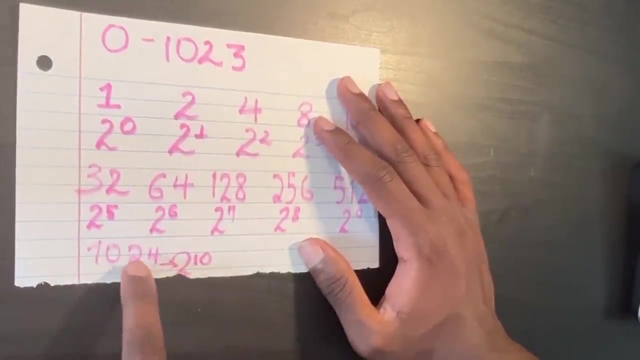 we have two, four, eight, sixteen, again to the power of zero, to the power of one is to the power of two, this to the power of three and to the power of four. this is what this is what this is. 10 bits. okay, so we stopped at 8 bits right here. this was what, 256. 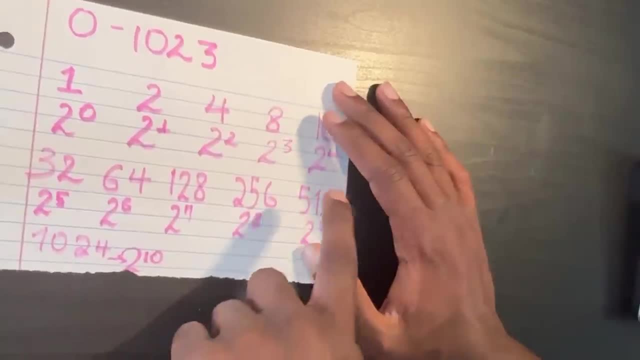 where we basically used for the analog right command. but this extends, and it can count to what? up to 10, 24, okay, to the power of 10.. that's why we keep receiving 10- 23. why do we keep receiving 10- 23? we're receiving five volts right here because i connected, uh, the five volts to the power of 10. 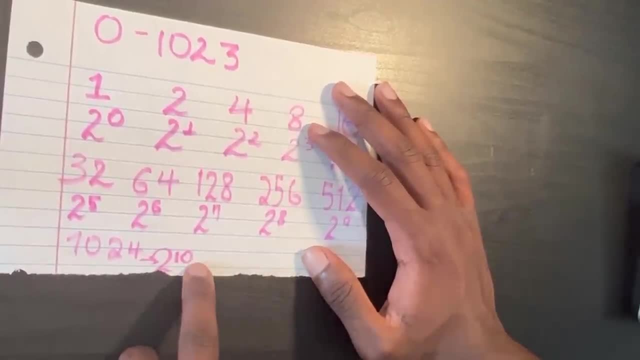 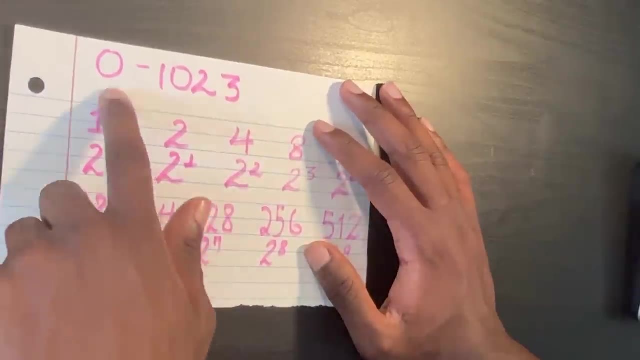 volt with the what with the analog pin. so i i expect the five volts. so five volt is what? 10 23? why didn't we say 10 23 instead of 10 24? because we start counting from what? from zero. that's one thing you need to know. so when you start counting from zero, what happens? it becomes 10 23, just like. 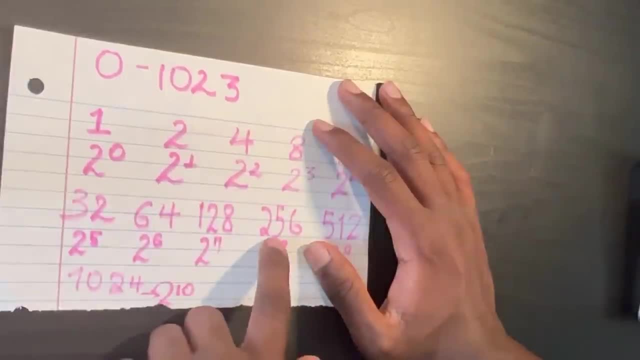 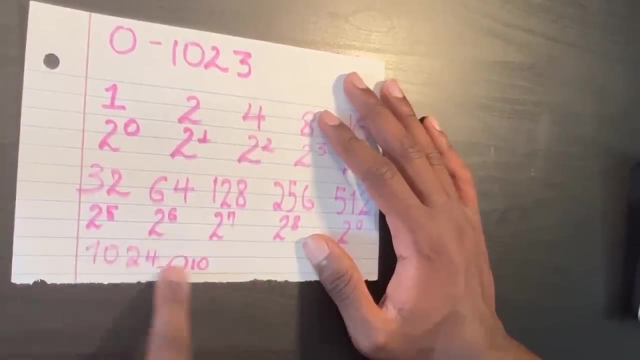 256. right, here we start counting from zero. it's going to be up to what 255, right? so 10 24 is what 10 24? it can store 10 24 items, but it can, because we still have 10 24. so we're going to start counting. 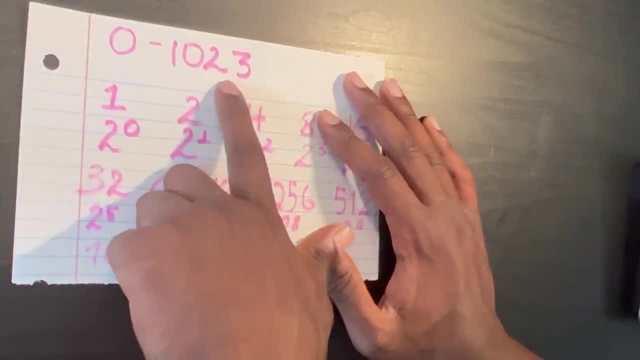 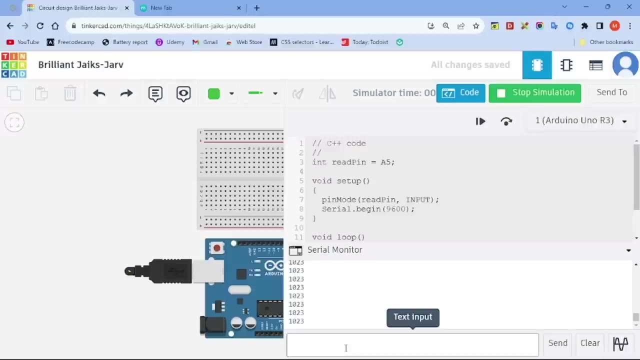 from zero. it's going to count to what count? to 10, 23, okay. so all right. so right here, we get 10, 23, basically meaning what five volt? we receive five volts, okay. so that's, that's what we basically are receiving. how about if i just um remove this five volt right here? okay, let me just remove this five. 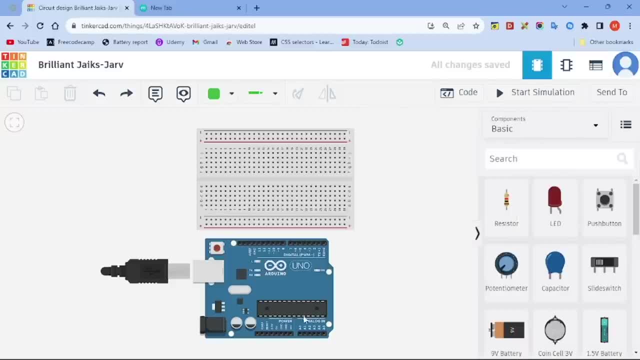 volt. let me stop the simulation right here. all right, let me just remove this five volt. i'm not going to connect this to the power of 10- 23, because it's going to count to 10 23. okay, so that's what we're going to connect the five volt anymore. so what i'm going to do is i remove the strength between the. 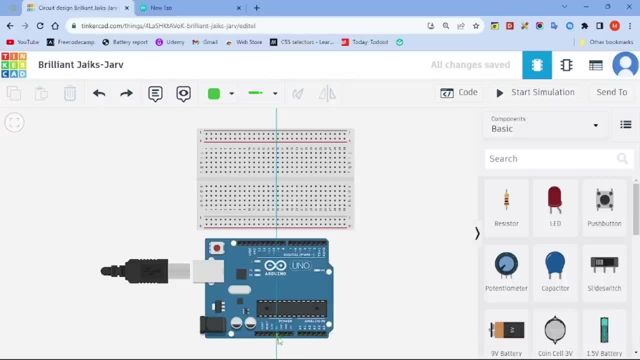 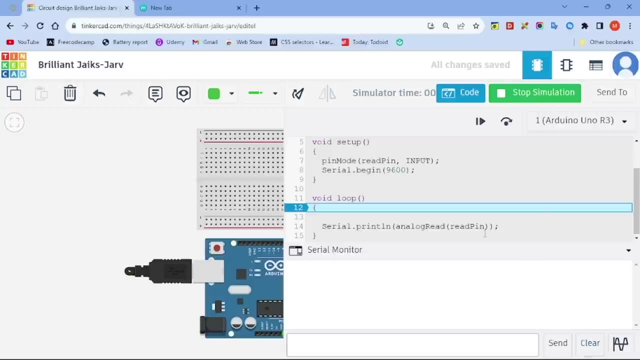 five volt and a5 right here. what i'm going to do is you know what? i want it to go to gnd. i want to connect the gnd with the a5. let's just do that, okay. so let me start the simulation right here. okay, let me start simulation. let me clear this one first. let me clear the serial monitor. let 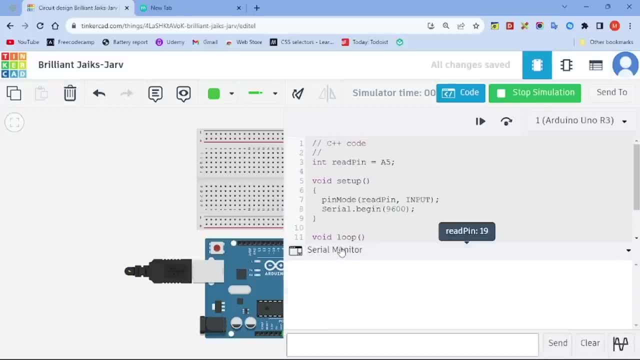 me just remove it and open it again. i should be doing that. i should fully remove it. stop the simulation, start it again. let me go back to the serial monitor. nothing's coming by, as you can see right here. nothing's coming back. can you guys see that nothing is coming by right here? 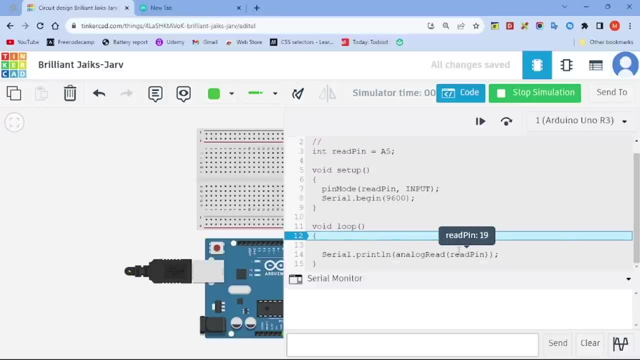 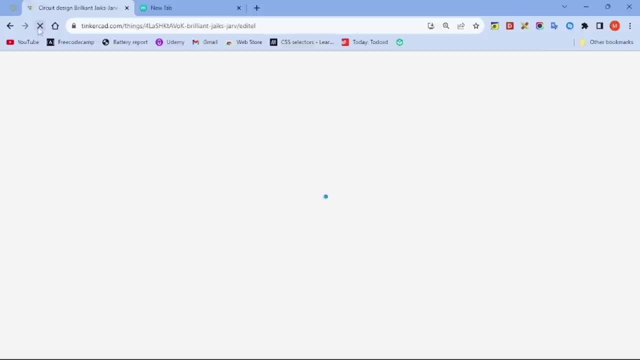 they're trying to read the pin, but i think it's coming by here. they're trying to use e5. let me just set clear right here, just to clear it up. but uh, nothing seems to be working. so in this case let me just uh Reload it. I think it's better to do it that way when we go through these errors of the serial monitor. 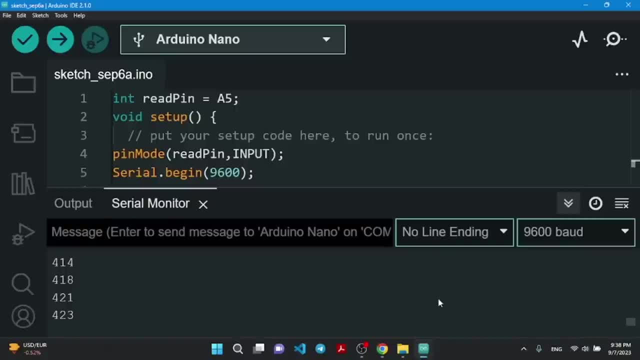 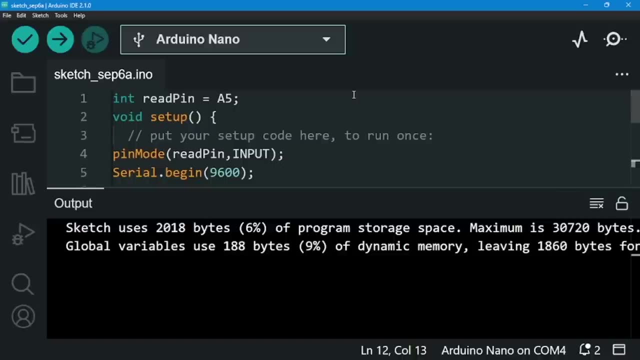 When I was using Arduino. what I could have done is you know I could have done- is what: Remove, close the window right here. I'm just going to do is clear it, And I'm going to do is close the window right here. I can do that. 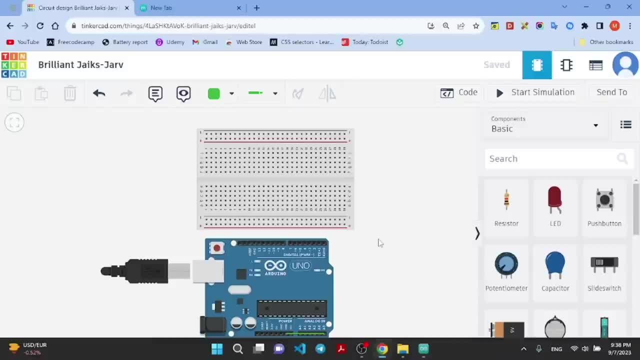 But sometimes, when the simulators again don't work because they don't fully mimic the physical world, I'm going to have to reload it because again it happens. OK, let me go back to code right here and let's go back to our serial monitor. 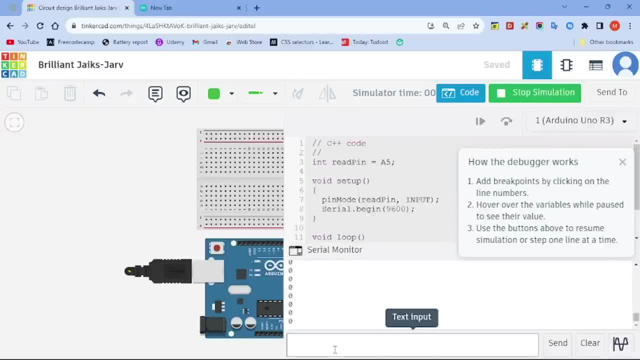 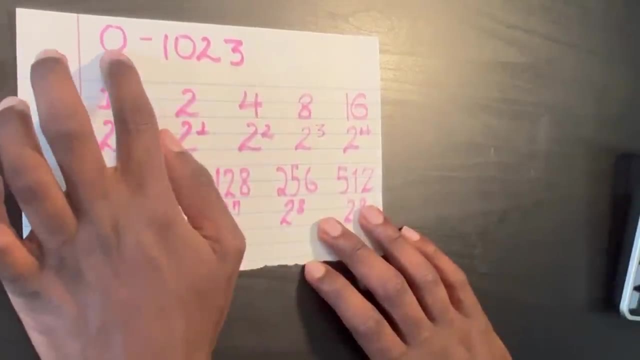 We keep receiving zero. when you connect to the GND pin, We keep receiving zero, zero, zero, zero and zero, like perfect pinpoint accuracy. I'm talking zero, zero, zero, zero. You can. you can see that right. When it's a five volt, we receive 1023.. When it's at zero volt, we receive what? 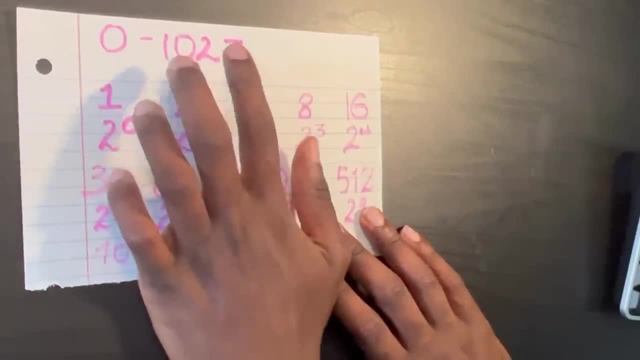 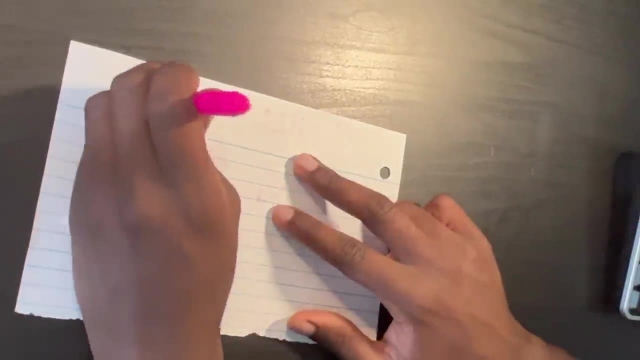 We receive zero. OK, so 1023 corresponds with what? With five volt. But we're reading it. When you're reading it, you're writing when we're using the analog write command. Let me just again for you to remember the when we're using the analog write command. 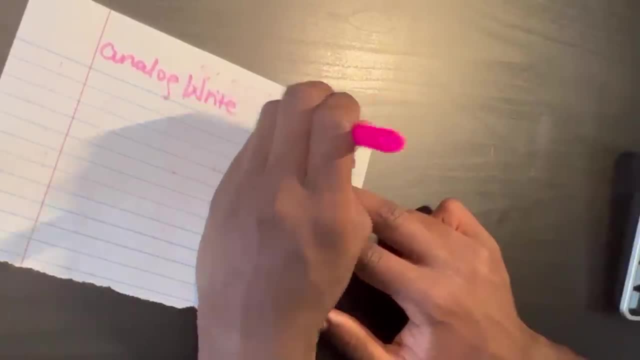 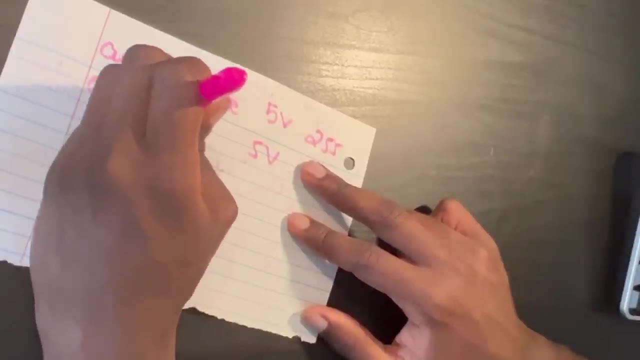 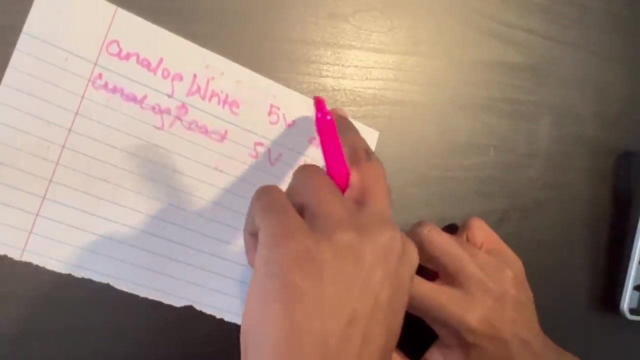 Five volt corresponds with what? Five volt corresponds with 255.. The five volt right here when we use analog read, corresponds with what? 1023.. I know it might seem a bit odd that we're using two different you know bit systems here. 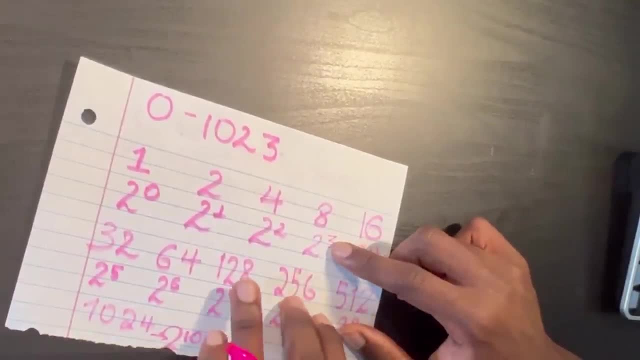 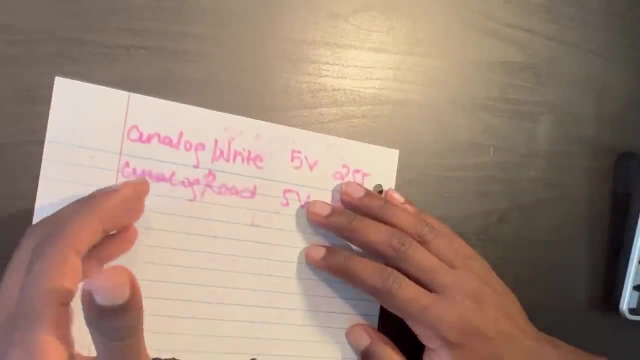 We're extending this to the power of 10 or we're just using to the power of eight for analog write. It might be, you know, it might seem weird or stuff, but it's just again convention. This is something that Arduino's people who built this decided upon. 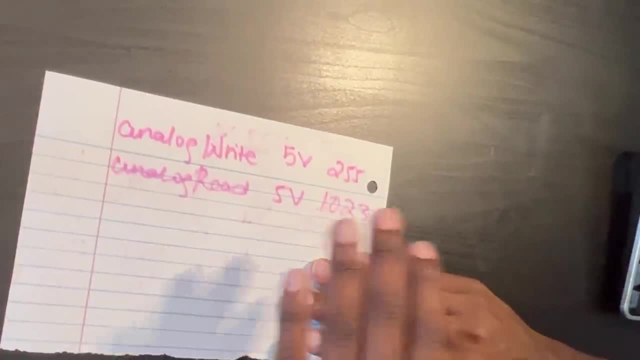 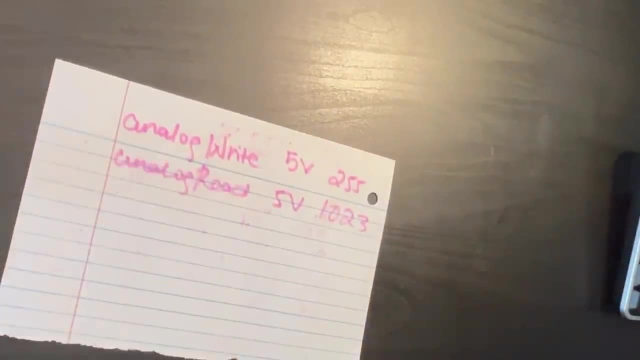 I don't know why they decided upon this, but as long as I'm concerned, it's going to be again 1023 for analog read and it's going to be 255 for analog write. OK, that's all you need to know. 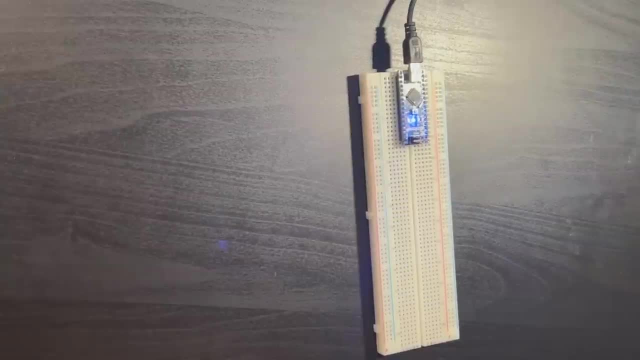 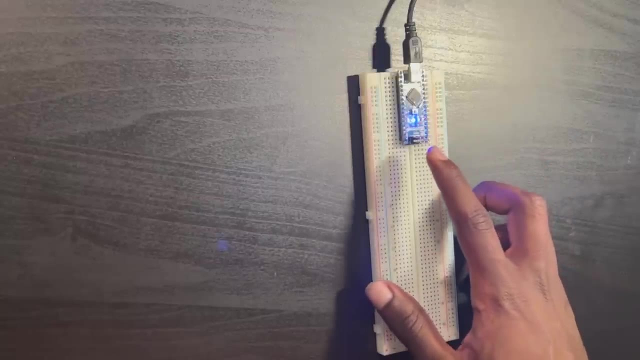 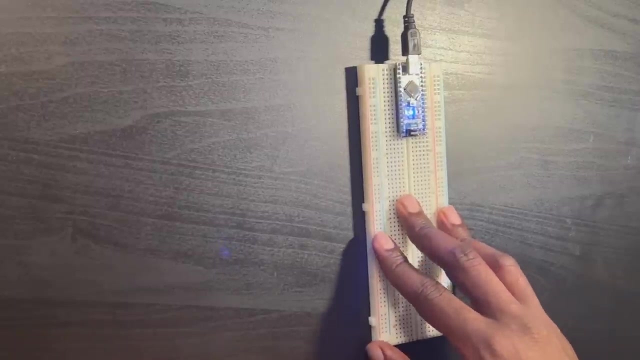 OK, so now we've worked with what We've worked with- analog pins, but we've not worked with a physical Arduino. We've been using simulators. OK, so let's actually work out with a physical Arduino and actually add a bit of a twist to it and make a good project. 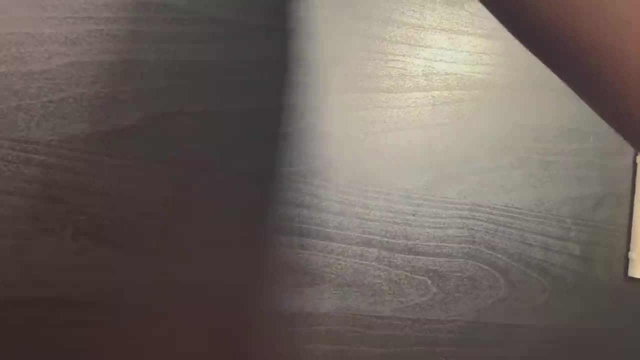 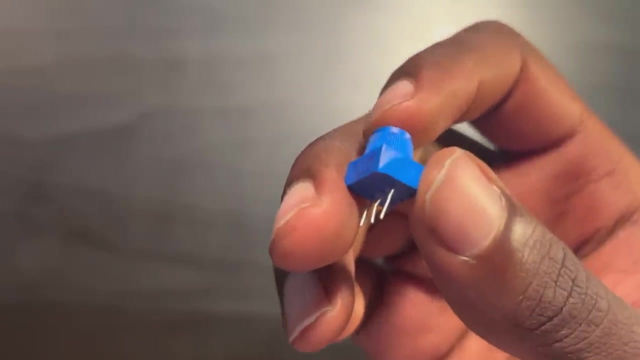 So I'm going to introduce a new electrical equipment right here, called a potentiometer, right here. If you look at it, it's blue right here It's called a potentiometer. It might be different depending on the kit you have. 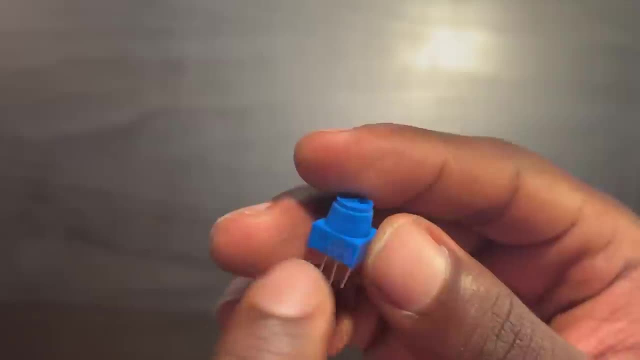 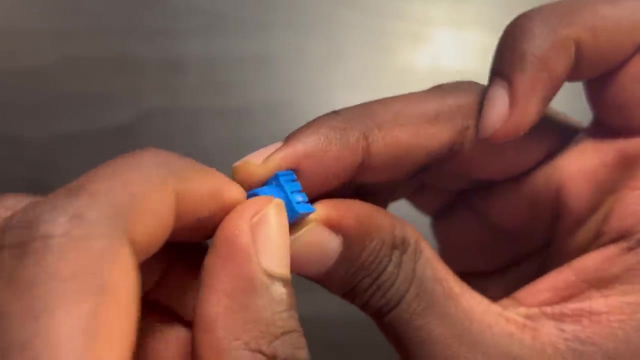 So it might even be black, It might even be long, But one thing you need to look for is three legs right here and an adjusting knob. So you have a knob that you can use to adjust. All right, So you have a knob right here that you can turn. 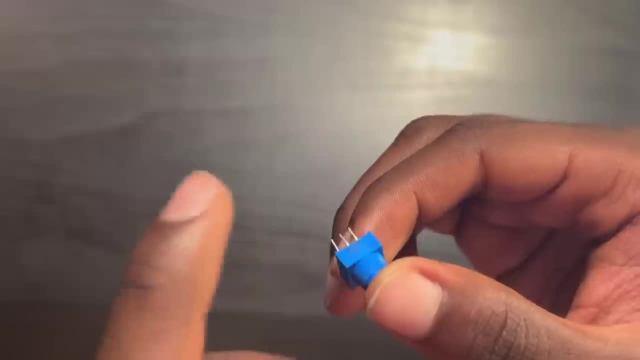 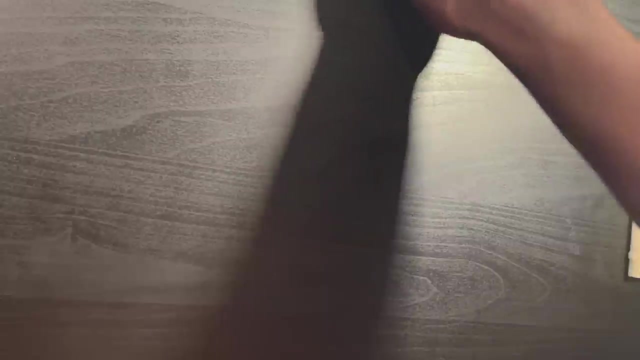 Those are the two things you need to look for in a potentiometer. So it might be different when it comes to yours, when it comes to your kit. So, again, check your label, All right. So check the label and check if it's a potentiometer. 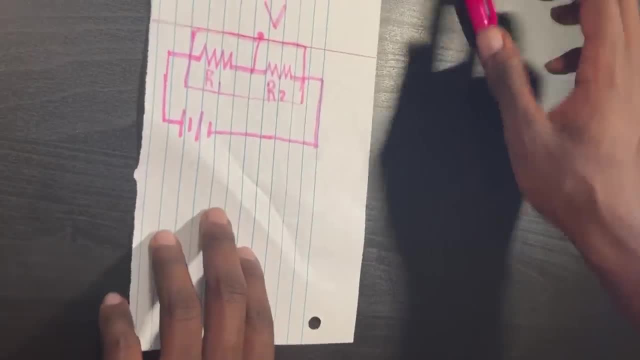 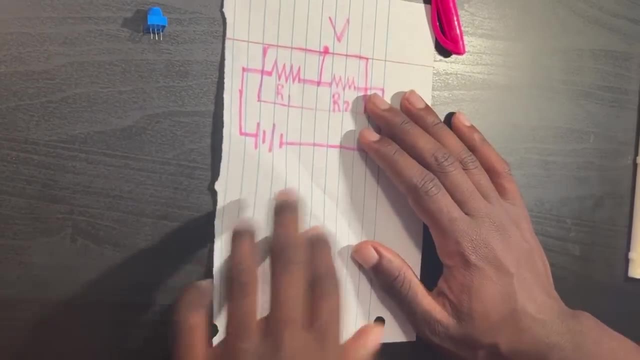 Check if it's a potentiometer or not. Okay, So what is a potentiometer? Again, before you know working with the component and stuff, we need to learn the science behind it. So let's check what a potentiometer is. 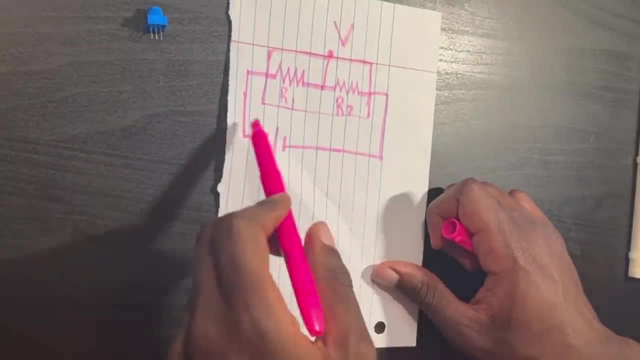 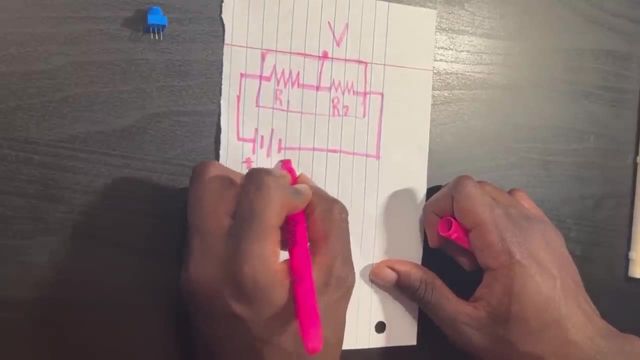 Okay, So we have the simple circuit here. It has a potentiometer here, And then it goes back to the negative terminal. It's the positive again. Again, this is the negative. The smaller one is the negative terminal. Okay, 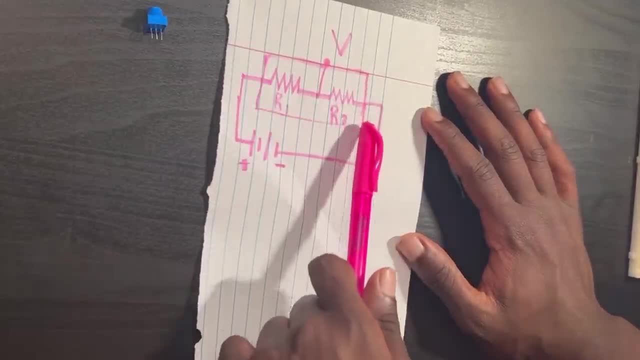 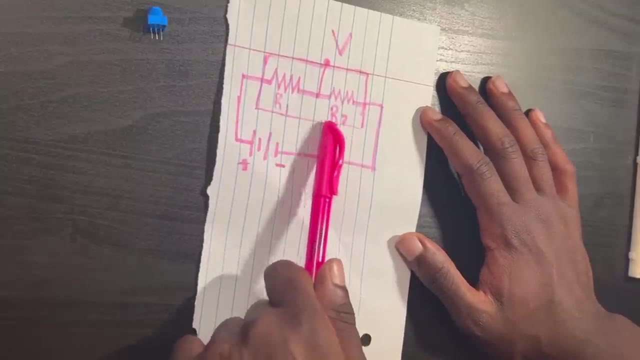 So the potentiometer. you can just think of it as what? As a box that has two, That has two resistors. here Let's call this one R1 and R2.. Okay So R1 and R2.. So just think of it as what? 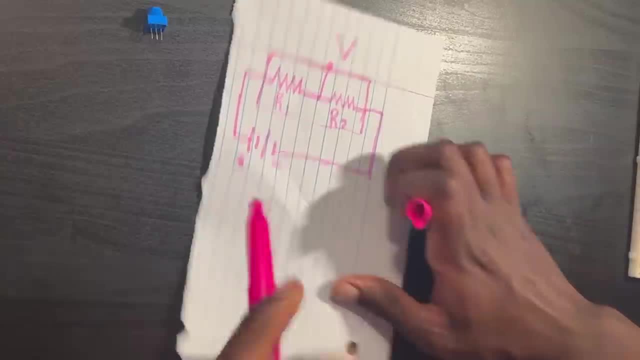 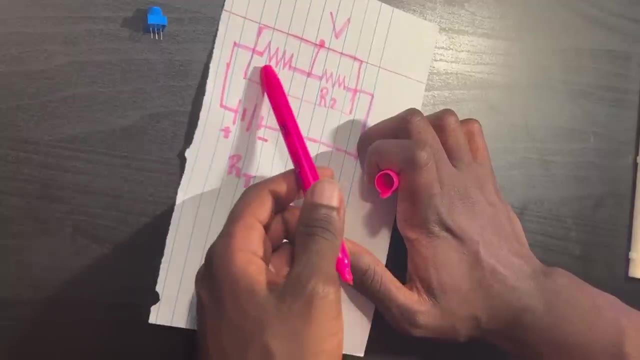 As a big box that has two resistors. Okay, So there's going to be what RT, let's just say it's the total value of resistance. here It's going to be what. Since it's connected in series, it's going to be what. 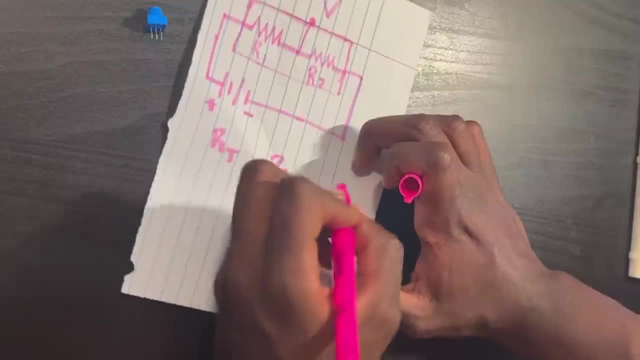 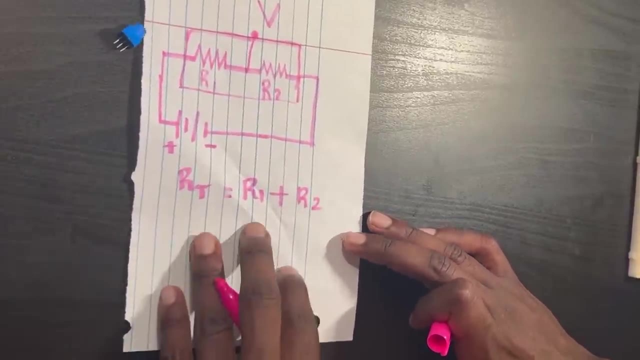 We're going to directly add them up. We're going to add them up directly. So we're going to say R1 plus what? R1 plus R2.. Because they're connected. what Directly? Okay, So that's all we're going to do. 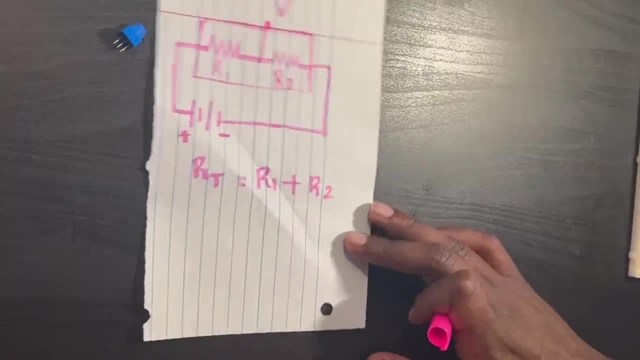 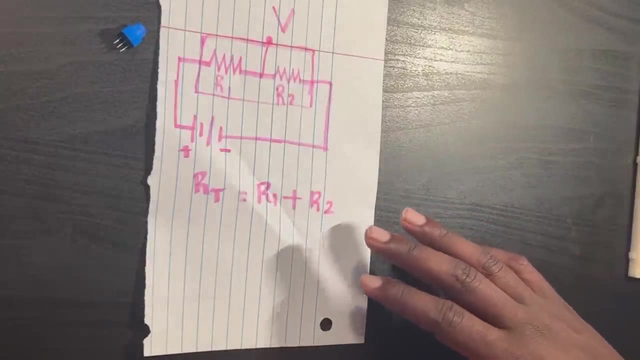 RT is what R1 plus R2.. So what does this let us do? What does a potentiometer let us do? Why is that? so that a potentiometer is very important than a. you know why is it different than a resistor? 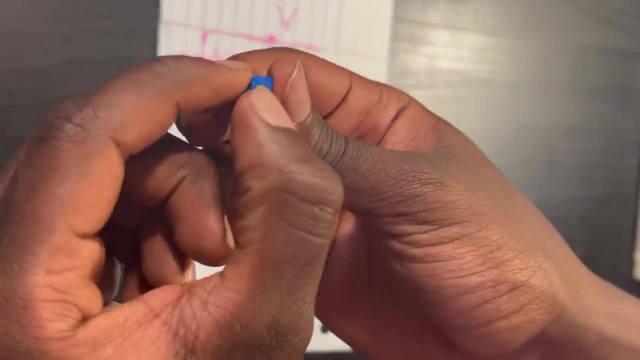 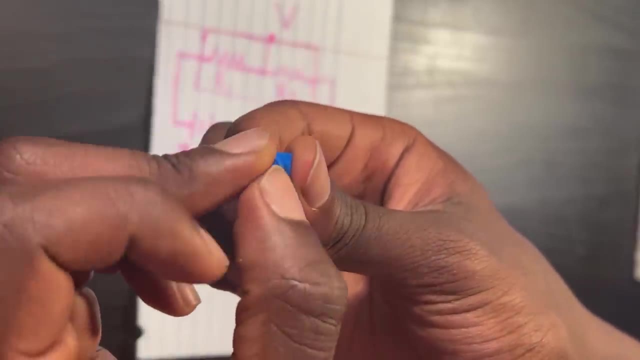 Think of it as a variable resistor. So when you adjust the knob right here, you can change the value of current, the value of volt that comes out of here. Okay, So you can adjust this so that what You can adjust the resistance- 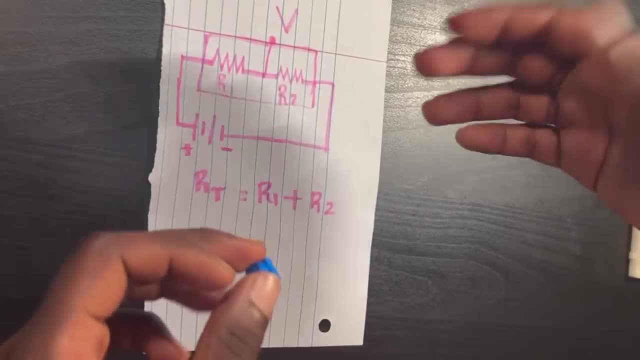 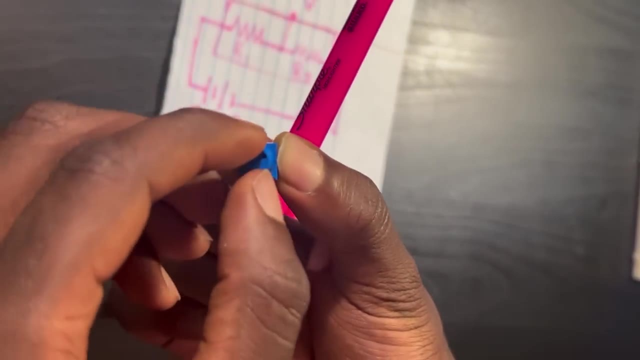 You can adjust the resistance here. So think of it as a what? As a variable resistor, Okay. So let's say, right here, I just put it all the way to the very end, to the very left. Okay, I'm just doing that right now. 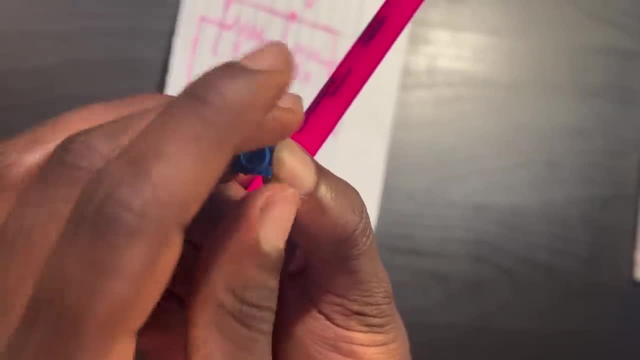 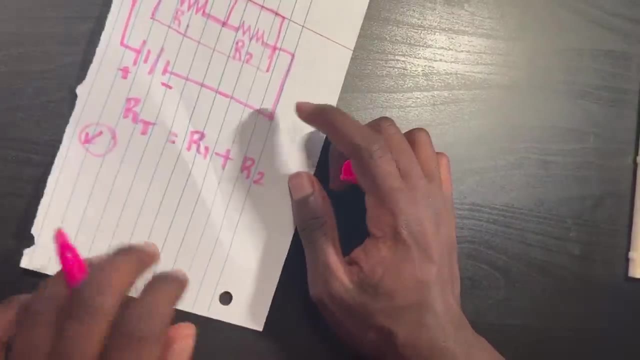 I hit the left, the very end. I can't move it further than this. Let's say I put it right here. What's going to happen is when I do that- let me just draw it right here- When I went, the very, very left, R1 is going to have a value of what? 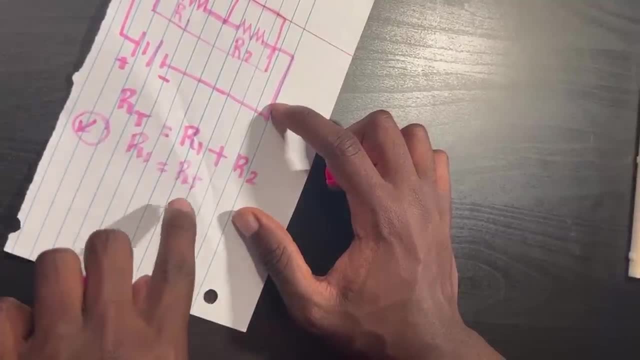 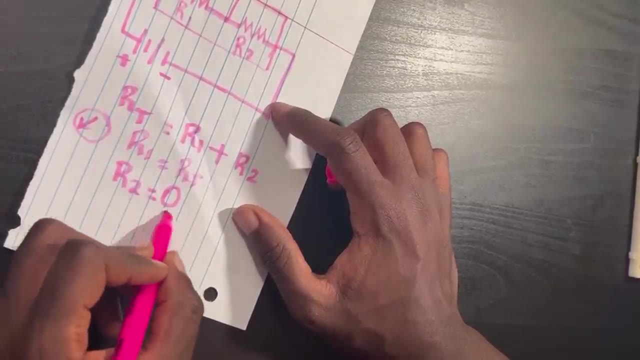 RT, RT, Right here, The total resistance, Okay, And R2 is going to be what R2 is going to be? zero Again. when I say zero right here, I've told you guys that there's nothing called as a. 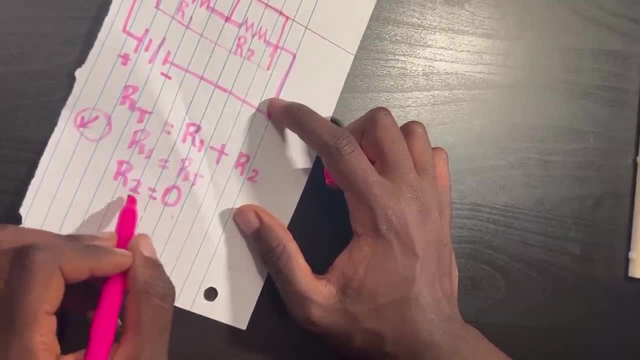 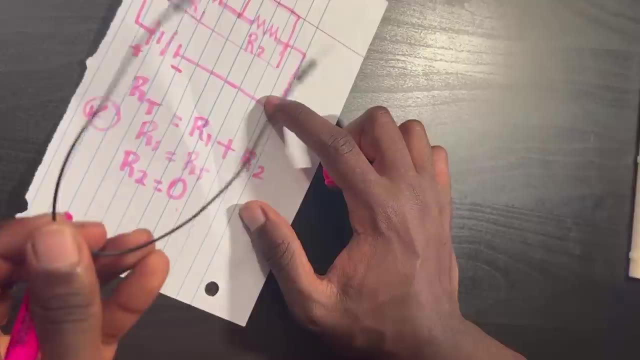 zero resistance, It's just a theory, Okay, So it's very, very small that it's close to zero, but it's definitely not zero. Okay, I haven't told you guys that even these connecting wires that are not you know, they don't serve. 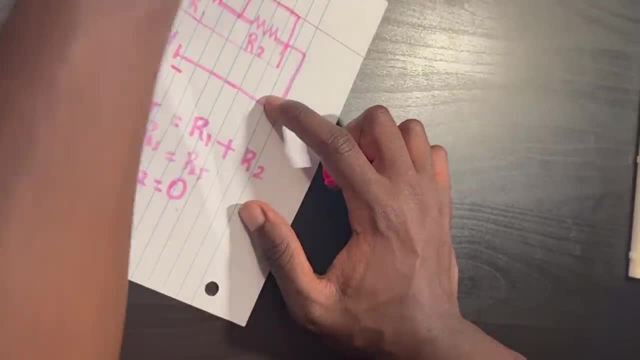 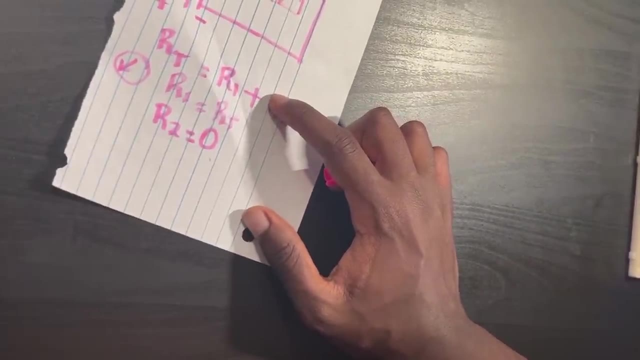 as a resistor, have what Resistance. So everything has a resistance, Even though it's what Resistance? It's very, very, very low, Okay. So in theory, it's it's zero, Okay. So, with that in mind, when, what happens? when I put it in the middle, when I put the 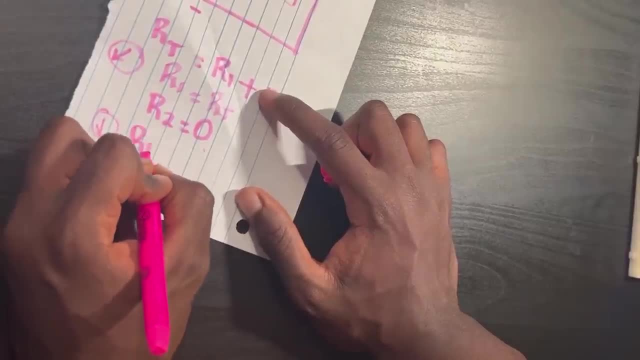 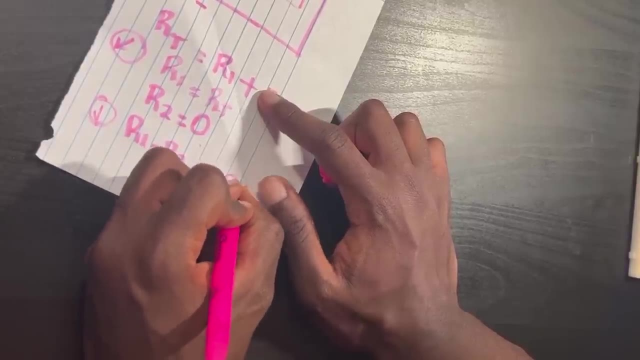 knob in the middle. what's going to happen is what R1 is going to equal to what R2, which is going to be equal to what. It's going to be equal to half of the total resistance, Half of what. 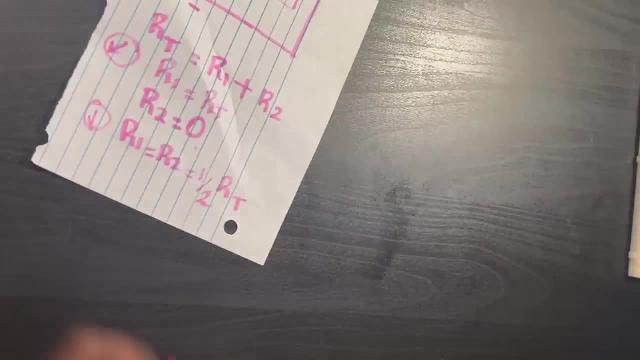 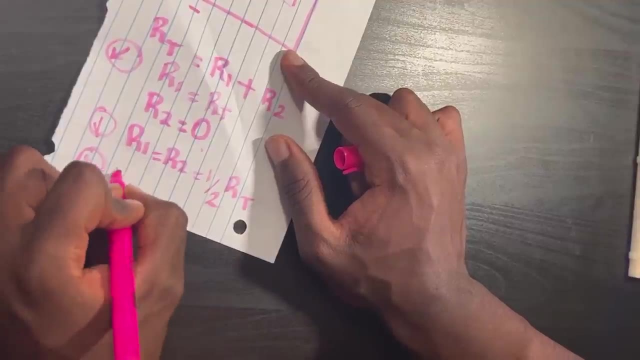 Total resistance. Okay, All right, Then what are we going to do? What are we going to do is basically go to the very, very right. So what's going to happen? So, in this case, what happens is R2 is going to be what. 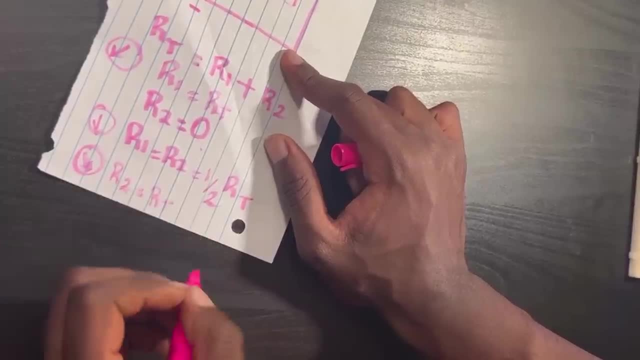 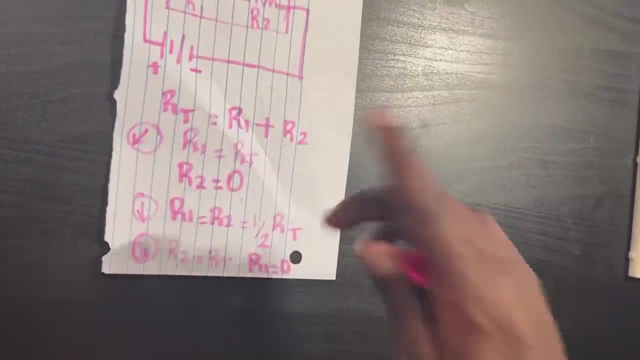 R2 is going to be RT, It's going to be equal to RT, while R1 is going to be what? It's going to equal to what? To zero. Okay, I just want you to keep that in mind, Okay. 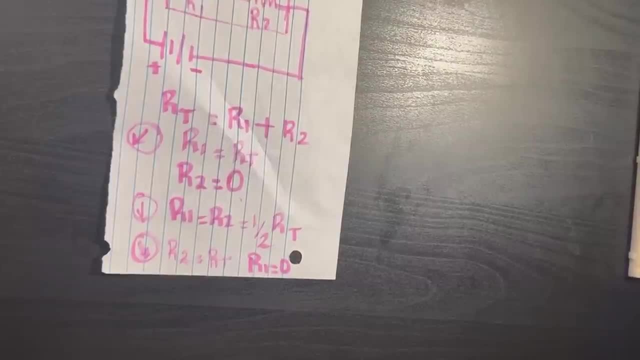 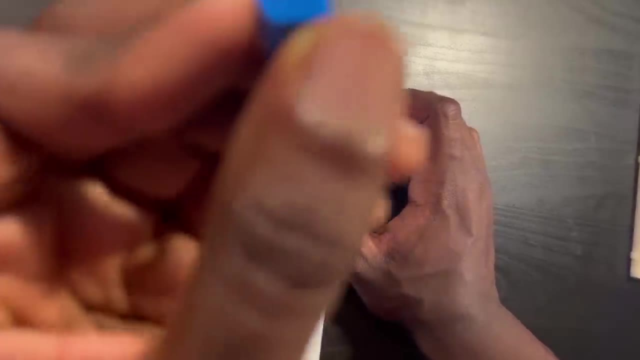 So right here, let me just turn this notification off. Okay, There we go. So right here we have this again, voltage out again. The voltage is going to be output right here. So we got these. Let me just go closer. right here. 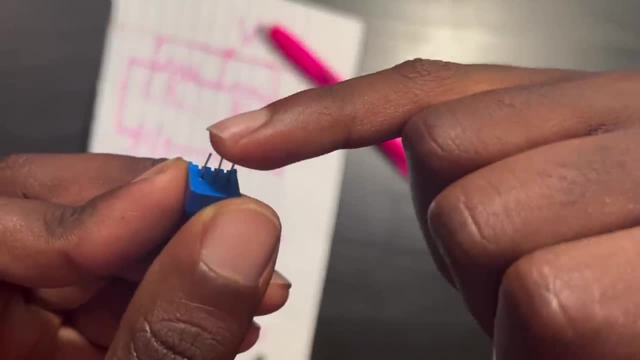 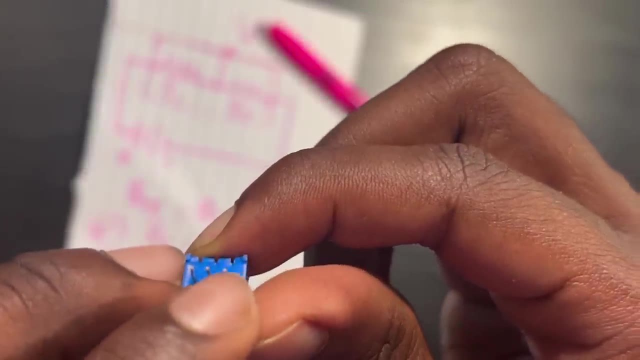 Focus on these. So you see those two. These are R1 and R2.. They're connected to R1 and what R2.. These are the final ones right here. Okay, The first one and the last one. they're connected to what. 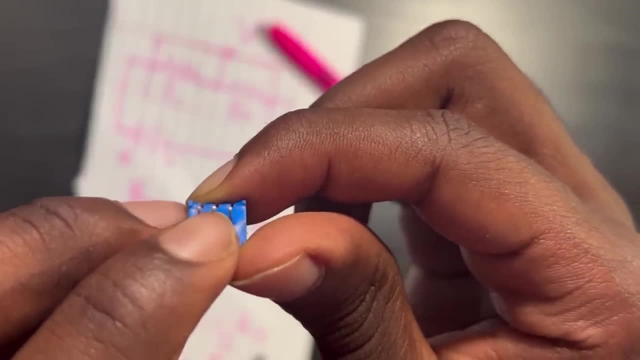 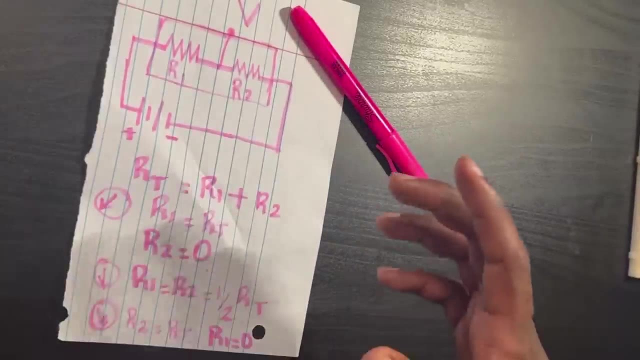 To R1 and R2.. And the middle one is connected to what? The middle one is connected to V out. This is going to be the voltage out. Okay, So with that in mind, let's just get started. So let me just put this potential here. 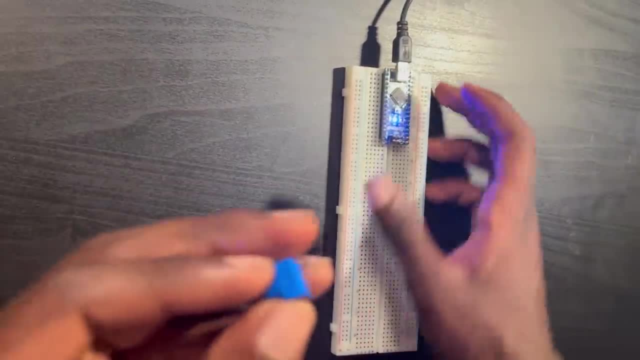 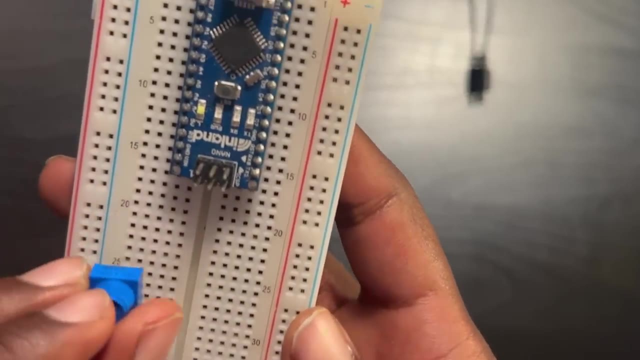 Potential meter right here. Okay, So again, when you put the potential meter, let me just remove my, let me unplug my Arduino right here. We need to what We need to put it across, We don't put it together. 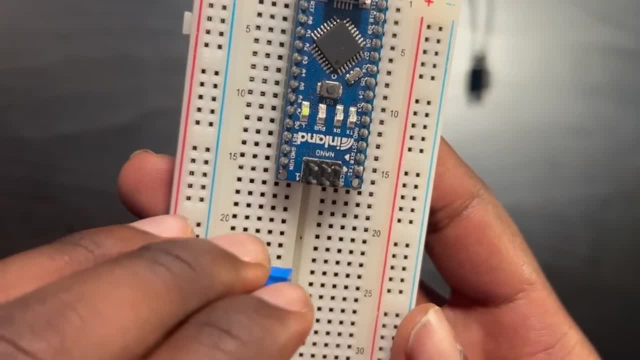 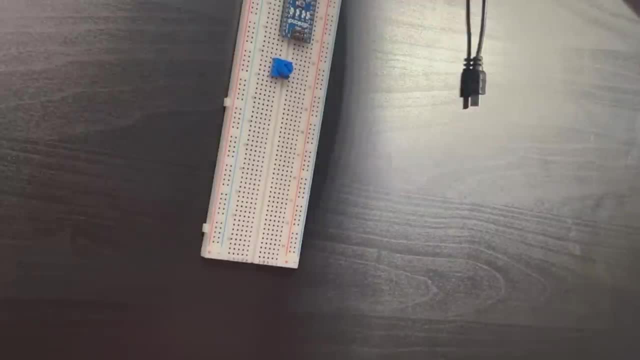 We don't put the wires together again, We just do it. what Across? Let me just put that across right here. Okay, You need to again look like it's facing the front, Okay. So, with that in mind, what I'm going to do is connect it to a five volt. 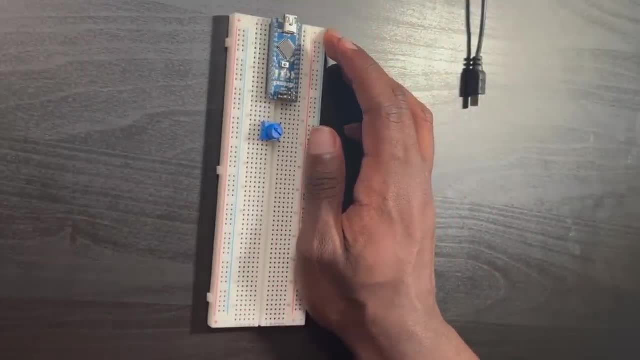 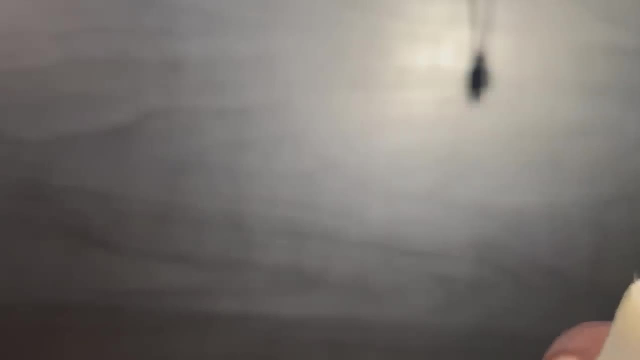 Okay, And we're going to use our analog pins to do what? To read the voltage out of here, Okay, So let me just do that right here. Let me just go on a five V right here, connect it to the, to the five feet. 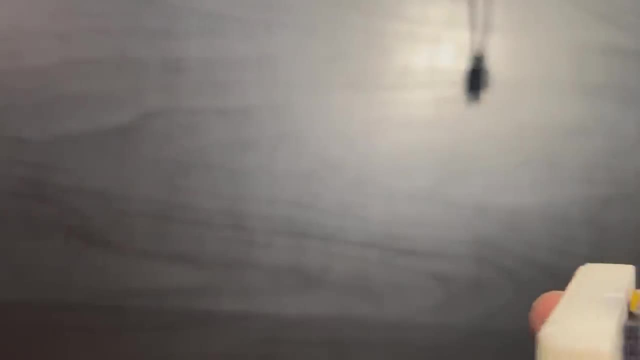 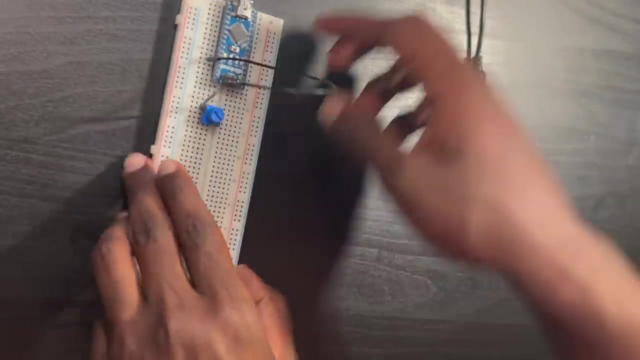 Okay, Let me just do that. Just go to the five V right here. Can't see it All right? There you go. I got it right here. I connected it to the five V with the black wire, And then what? 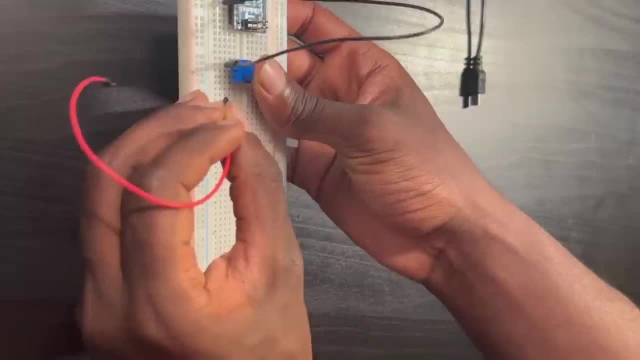 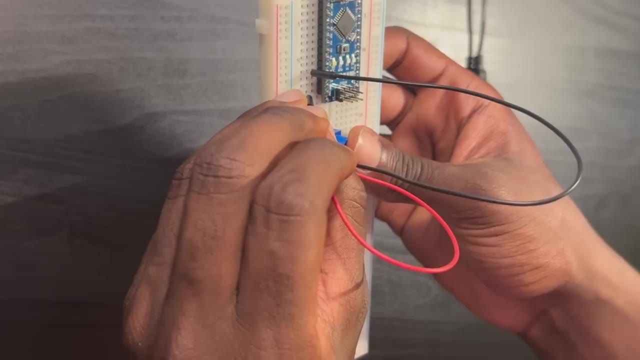 Let me just connect the third one right here, The third one, the third leg, the last one right here with the. what With the GND? Let me just connect them with the GND right here. Boom, I did that, And then, finally, I'm going to need an analog voltage again. 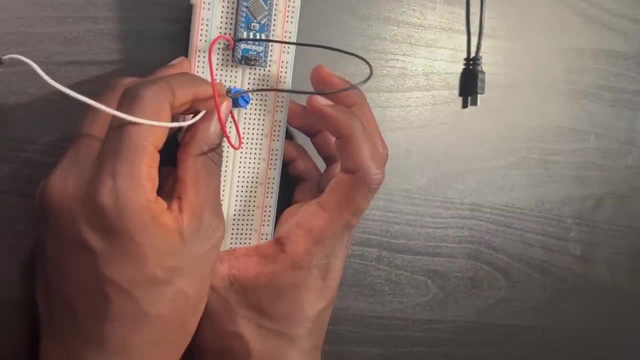 The voltage that I'm going to be reading off of. I'm just going to put it in the middle, in the middle pin, right here for you to see it in the middle pin, Okay, And I'm going to put it at a five. 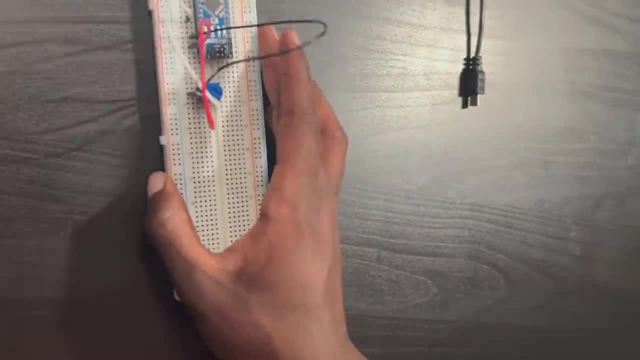 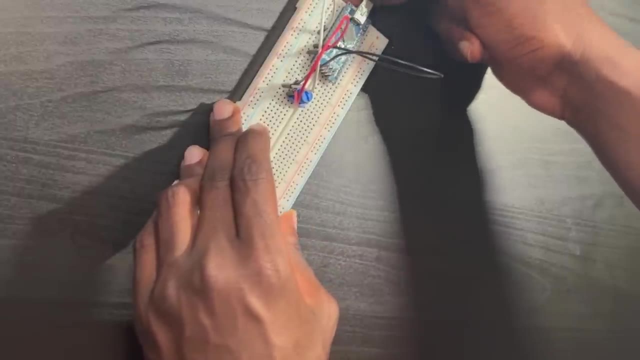 So I already have this code with it, As I read it earlier. So what I'm going to do is it's already uploaded, So I'm just going to run it. Okay, You guys can look on my screen if you guys remove the code or not, but I already have. 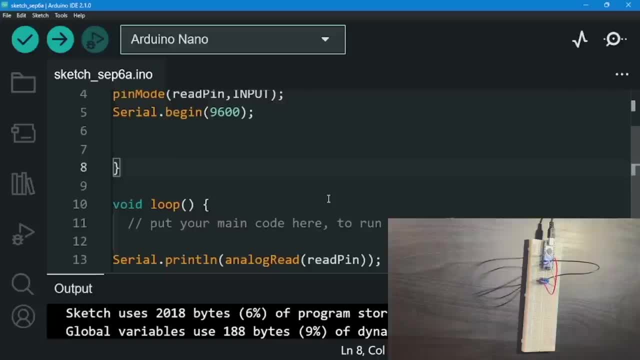 it. Okay, So let me just upload. It's already uploaded right here, So let me go over to my screen right now and let's open our serial monitor. Let me go to my serial monitor right here. Let me just make this a bit taller. 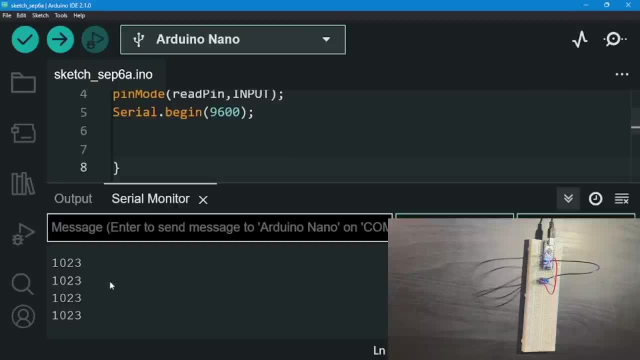 All right, There we go. Maximize it. It's 1023.. It's outputting 1023, 1023, 1023.. So let me just adjust it right now. Let me just adjust it a bit. Can you see it's going lower. 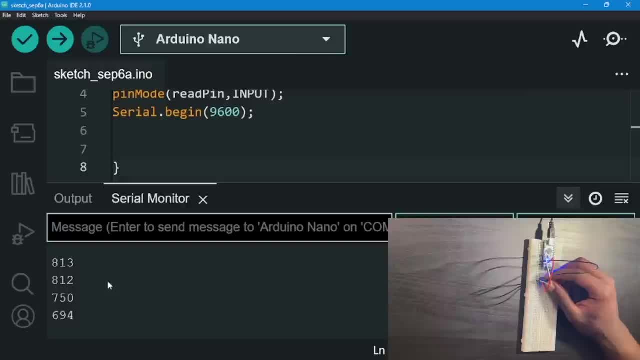 It's going lower, lower, lower right now. Let me just try to put it in the middle, roughly in the middle. All right, It's going lower right here. It's roughly in the middle, bit. Okay, It's roughly in the middle right now. 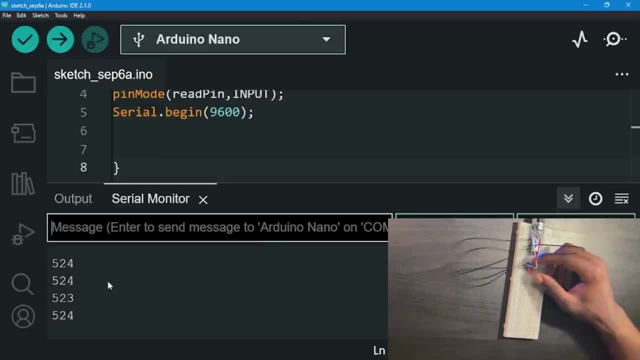 I put it straight, So it's roughly in the middle, And then let me just adjust it until it goes to zero. Let me just adjust it all the way down. Let me just do that. You see that we're changing the what. 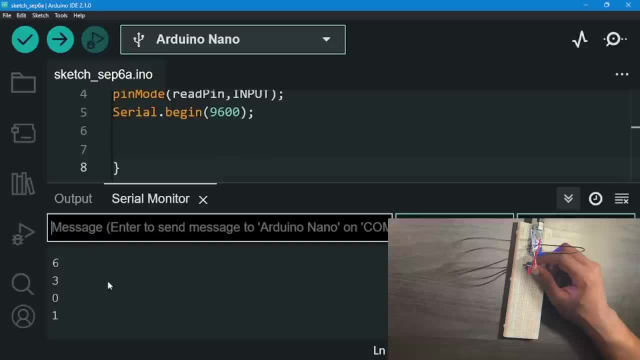 The voltage value coming out right here. Can you see that We're going to zero? We don't get to a true zero right here, But we get something that's very close to zero. What is going on is we're getting values like zero, point something. 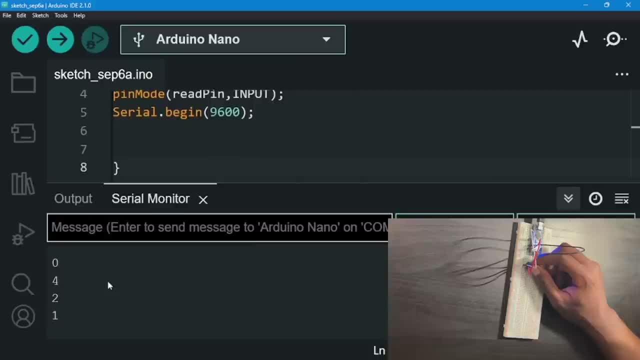 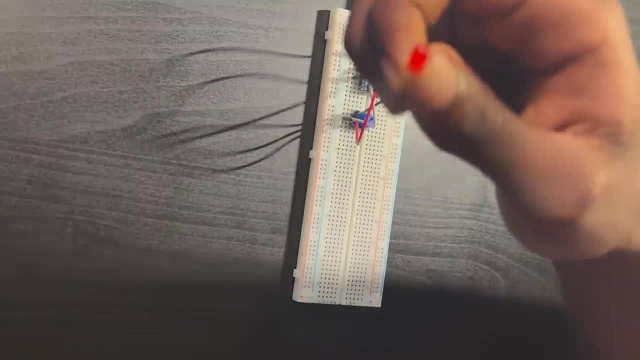 And sometimes it rounds it up to one, Sometimes it rounds it down to what To zero, Okay. So, with that in mind, something that actually can make this more interesting is what Putting on an LED. So what I'm going to do right here to put on this LED actually makes things interesting. 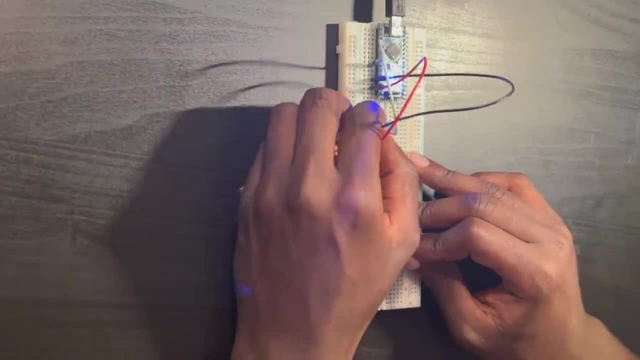 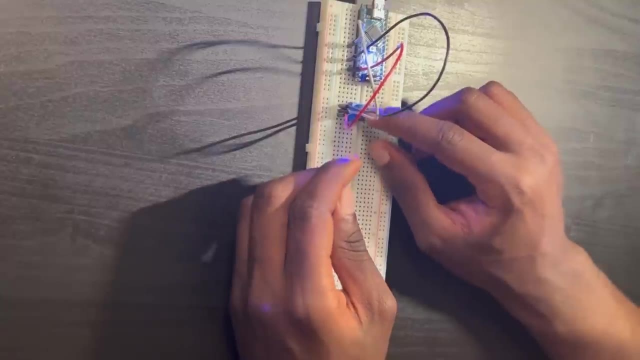 Let me actually move this a bit, because this is taking too much space. Let me just again move it to the very front, This line right here. That's all I'm going to do. I'm not going to change anything, because this is going to take a lot of space. 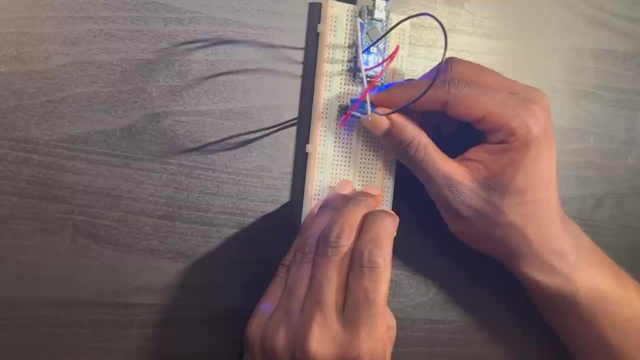 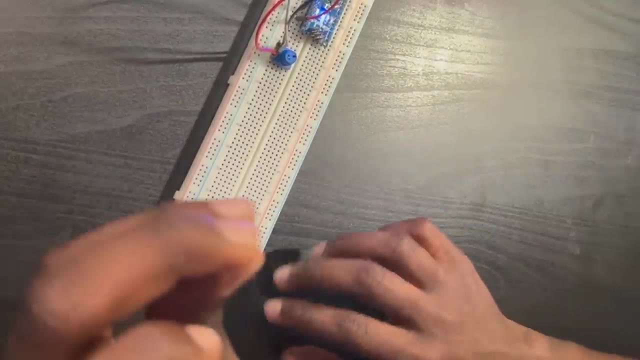 Let me just go and put this as close as I can to the wires. It just takes a lot of space. Okay, I have one space right here, So I'm going to again connect the positive terminal of my LED right here. to what? 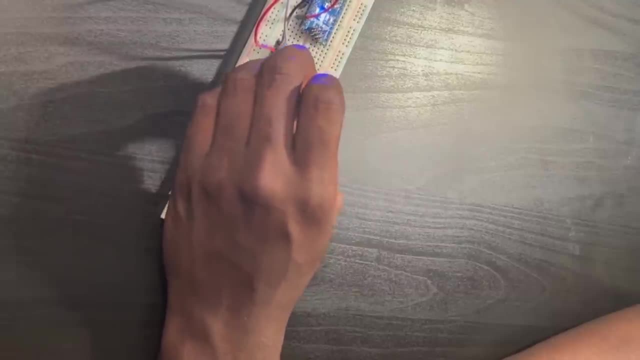 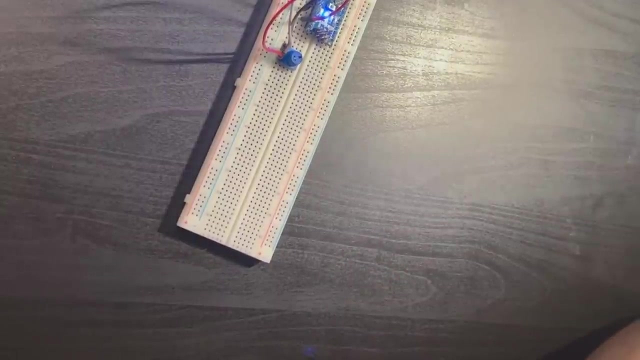 To one of the resistors, R1 or R2, whatever you want to pick. I'm just going to connect that, And then what? And then I'm going to connect the negative side of it to what? To the GND. 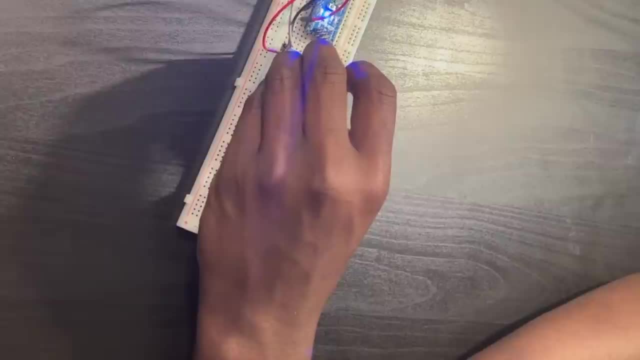 So I'm going to need to do that. Let me just do that. Okay, Let me just connect these two pins. I'm not connecting the middle pin, I'm connecting the positive, the one, the black one and what? The red one. 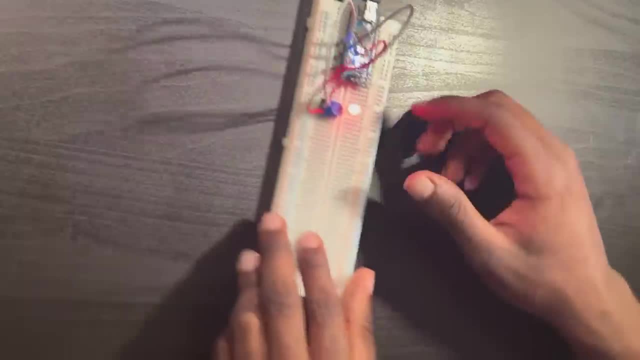 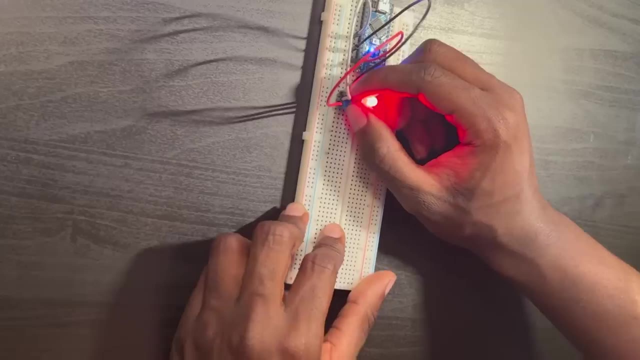 Okay, I'm connecting those two. Let's see what happens when I try to adjust the knob right here. Let me just try to adjust the knob. All right, Let me just do that. It doesn't work. Why is that so? 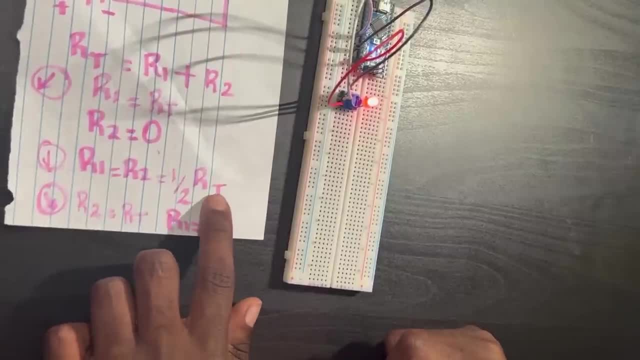 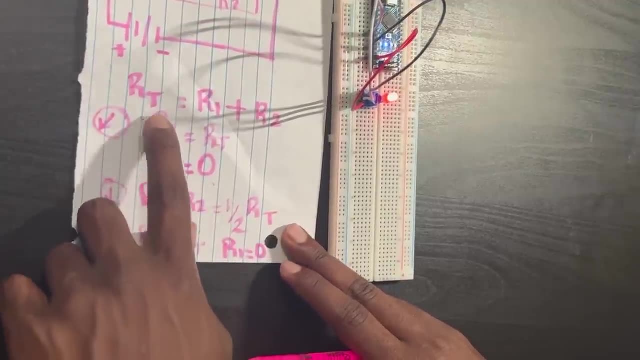 One thing I need you to understand. The potentiometer says what RT is fixed. okay, RT is always fixed. What is changing is always R1 or R2.. The value of R1 or R2 is changing, But RT is what. 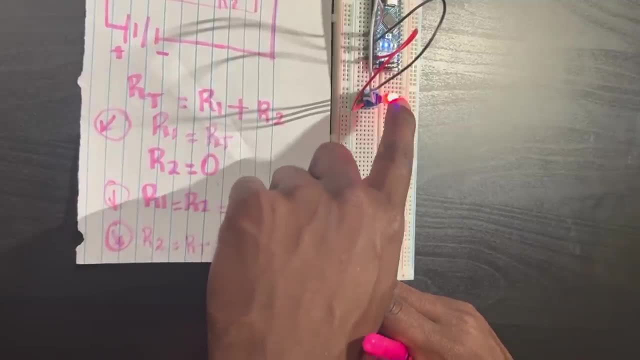 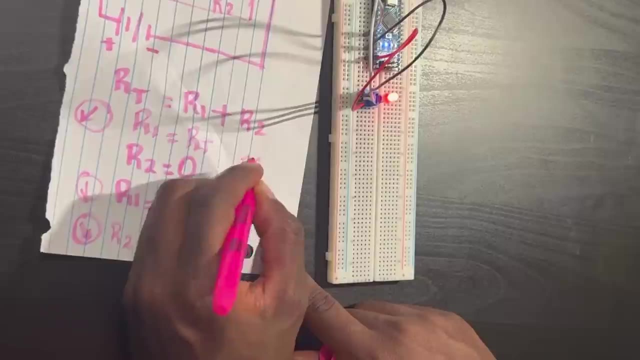 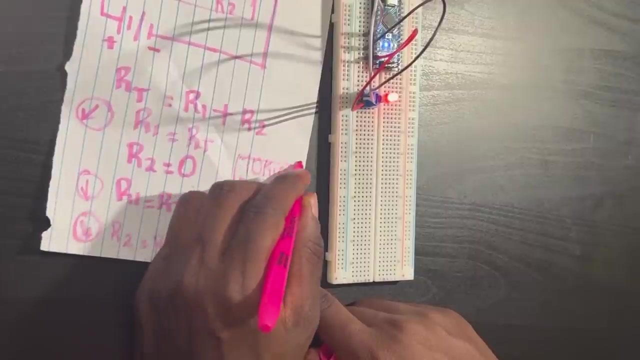 It's always fixed. Okay. So when I'm going through the whole resistance right here, RT is what It's always fixed in the potentiometer. Right now, my potentiometer is what? 10K ohms? And it's going to be written on your potentiometer or at least at the label of how much resistance it has. 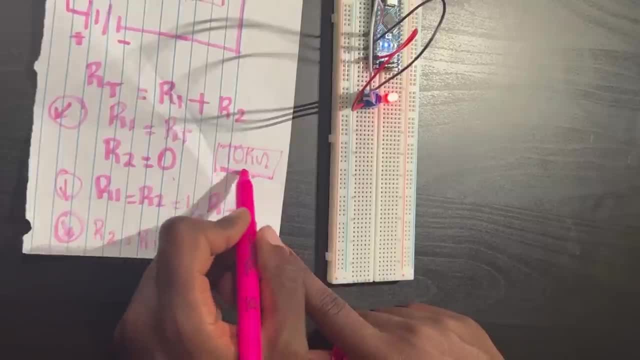 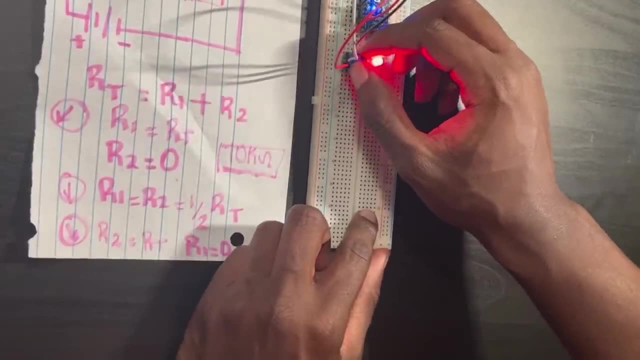 Okay, So it's going to be the total resistance Minus 10,000 ohms. Okay, I want you just to know that, But it's going to be written for you, All right. So with that in mind, if I just again run this over again, it won't work. 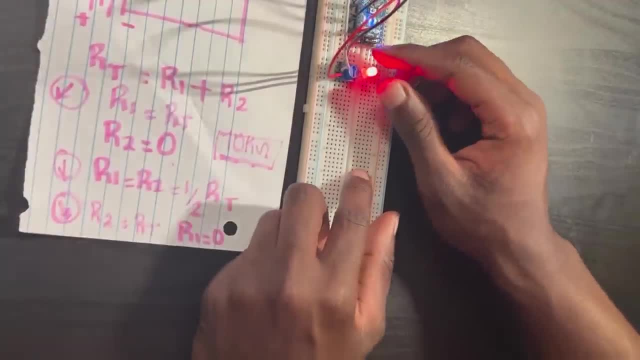 So what I need to do is what I need to go to the middle. So let me just do that. How do I do that? I connect the GND again to what The GND is- the red pin, if you remember. 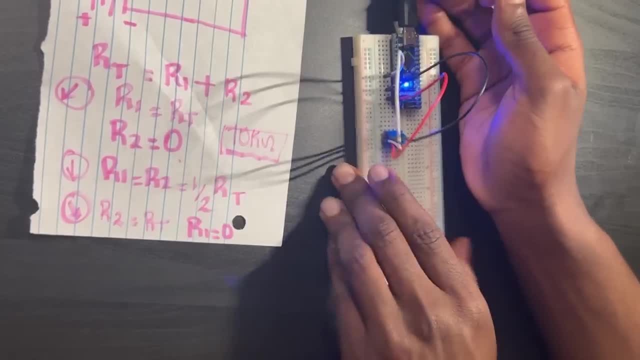 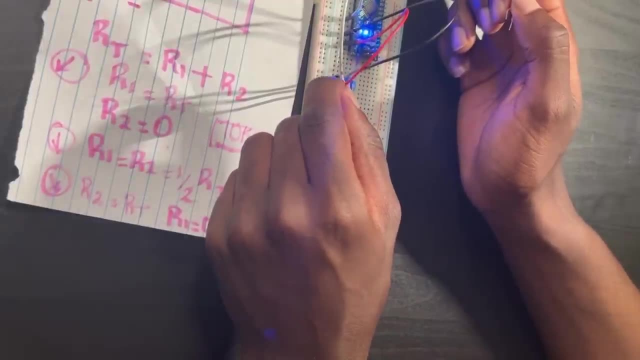 The GND is what The GND is connected to which pin? Let's just remember that The GND is connected to the red pin. Okay, It's confusing me a bit, because the red pin is supposed to be connected to 5 volt as a standard. 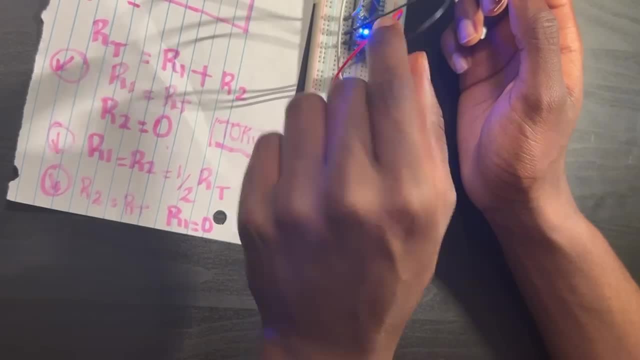 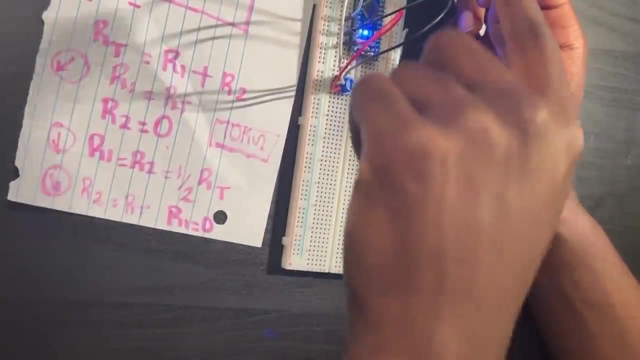 And like the black pin is supposed to be connected to what? The GND? That's the standard again. Again, it does not change anything, but it's like a standard between electrical engineers. But I just, you know, I rushed over it and just changed the color. 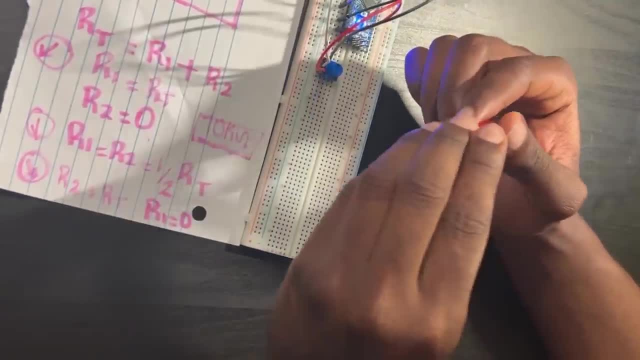 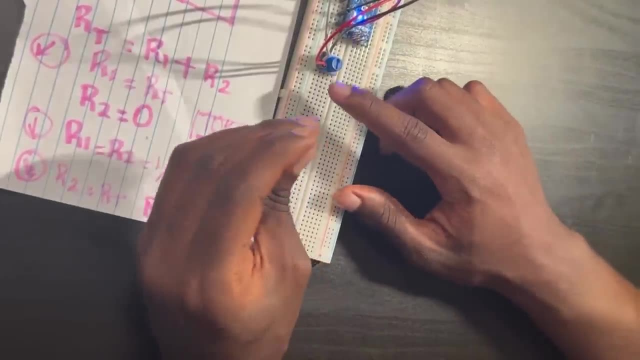 So it got me a bit confused. All right, So let me just connect the positive side to what, The positive side to the middle pin. So I'm just going to connect the middle one and the negative side of the LED to the what. 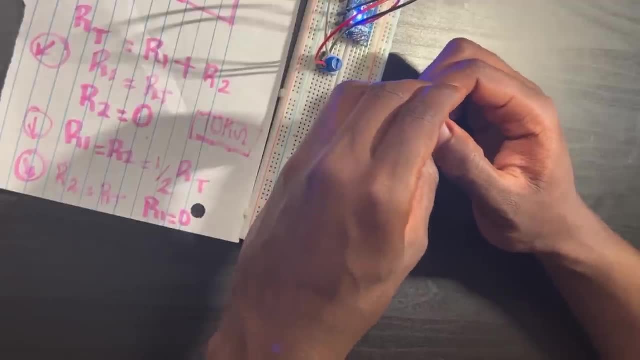 To the red one To the red one. So let me just do that. It's crossing over. I don't want it to touch each other. That would be bad. I don't want that to happen. Okay, There we go. 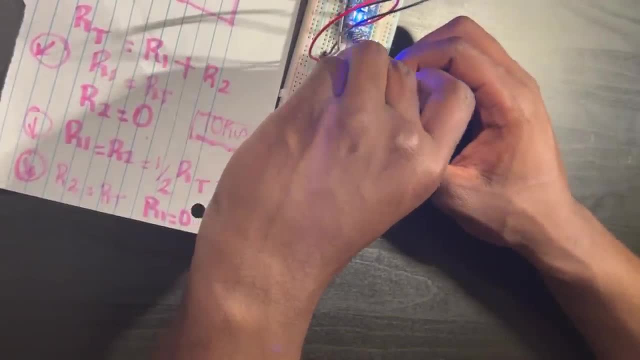 No, let me just go tighter right now. Tighter right here, Right, I think this is the one. All right, So now let's try to adjust it. Okay, Let's adjust our knob. Can you see it? It's dimming slowly, slowly, slowly. 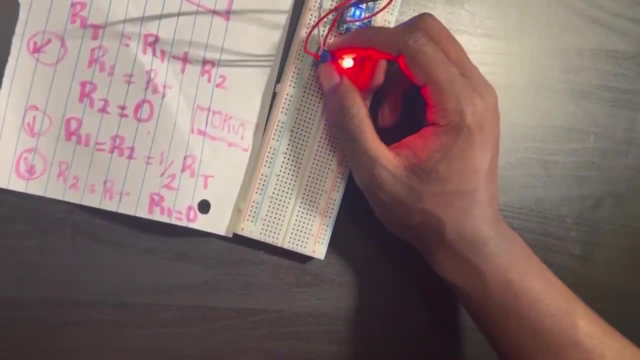 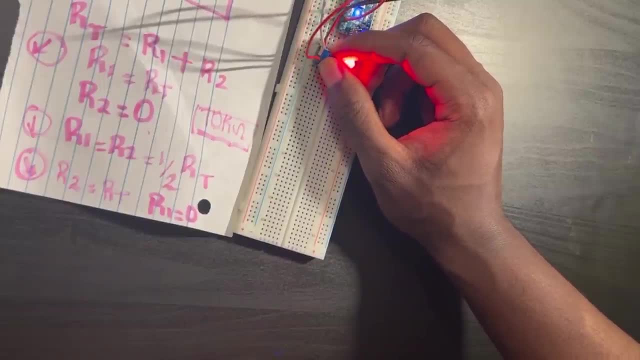 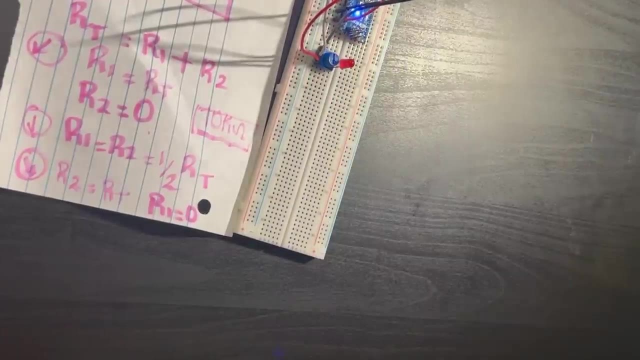 It's dimming. It's dimming especially when it's going slowly. You see that We did that. All right, That's beautiful. Now it looks nice, But before, finally, we actually finishing up our project, where we are going to do is 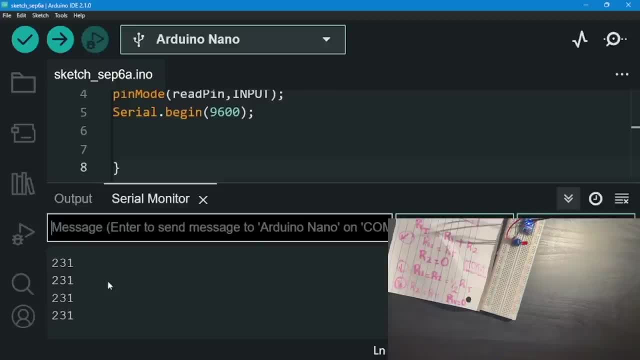 what I want. to look at the serial monitor right now it's outputting 231, 231- some value. Let's just change this to. what Let's just change is to something that makes more sense to us, that has some something. 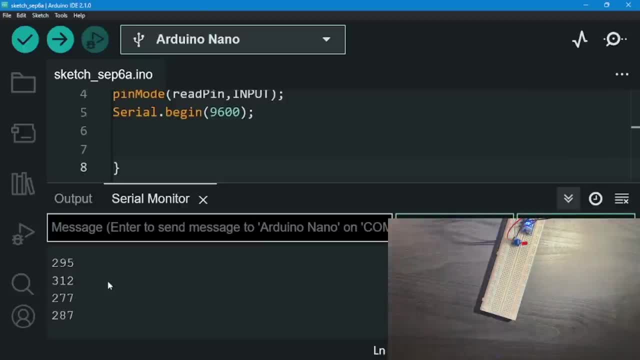 that is what That is a value to us. again, I don't want it to show to between 0 and 10, 23.. I want it to show what I want it to show: zero to five volt. So what I need to do right here, it's quite simple. I need: 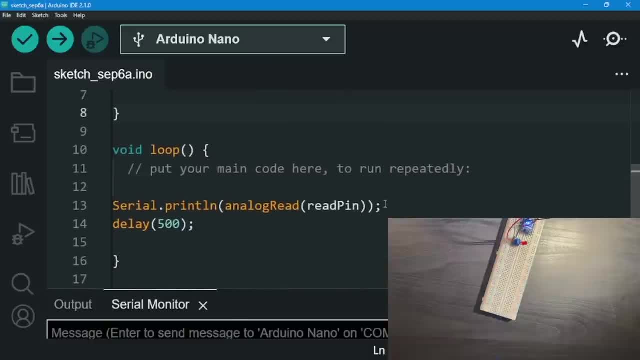 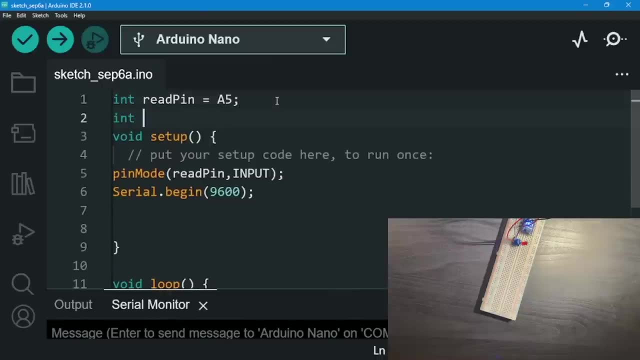 to do some bit of math right here. So what I'm going to do is what I'm going to say. you know what? Let me just set up a value right here. I'm just going to say int, I'm going to say calc value. 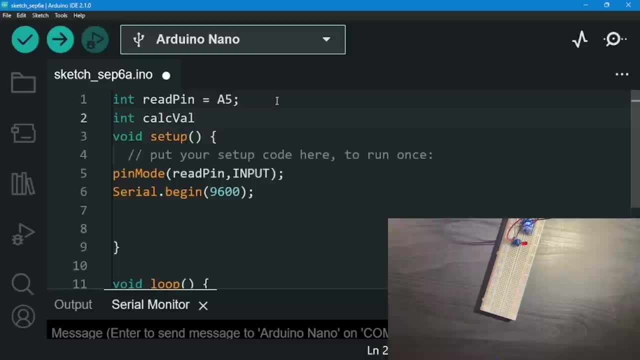 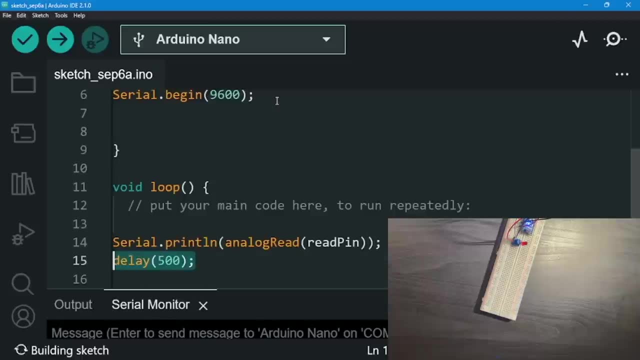 because I'm going to what? Calculate it? So I'm just going to say calc value, And so what? Let me just set it to zero for now. Okay, Calc value, and what? Let me just? okay, there's a delay, right? 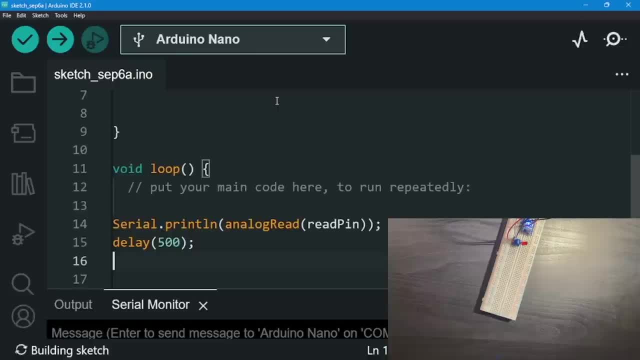 here. Let me just go beneath that, And what I need to do is what? Just set up the calc value. right here, Calc value is set to. what I'm going to say is what It's going to be. what It's going to be. 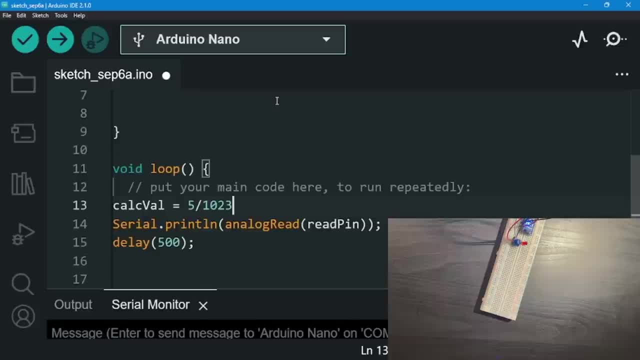 five divided by 1023.. I'm going to divide that. Then you're going to what? Multiply it by what? I'm going to multiply it by what. I'm going to multiply by the analog lead. I got that wrong Analog lead- And I'm going to say, okay. 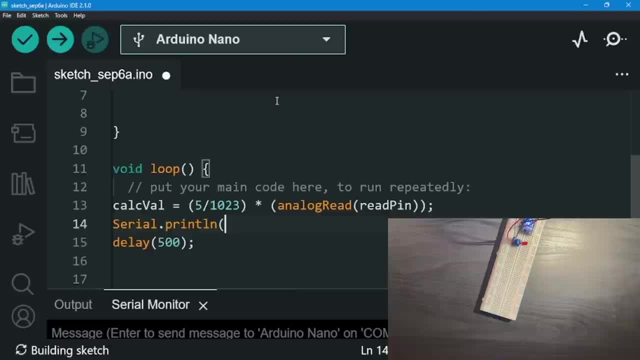 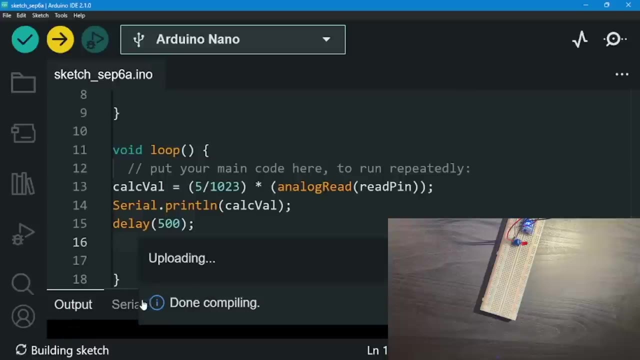 Just multiply it right here And I'm just going to say: calc value. Okay, There we go, All right, So what I'm going to do is upload it right now and let's see what happens. So let me just upload it right now Again. my serial monitor is it off? There we go. Is my serial monitor. 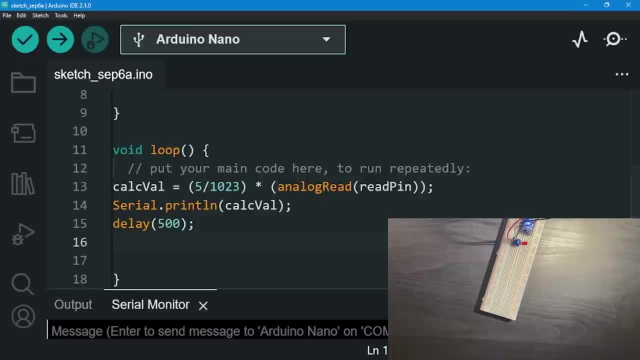 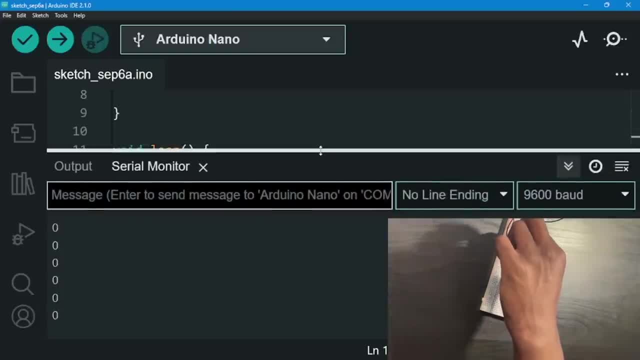 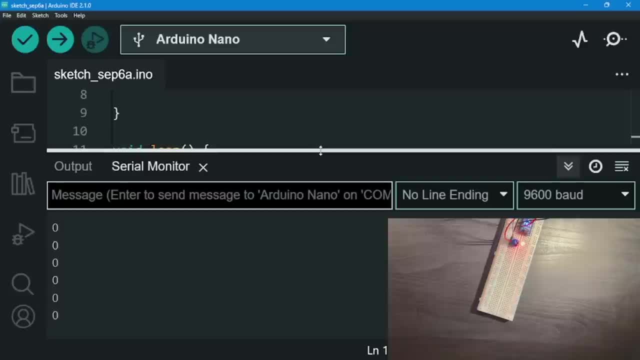 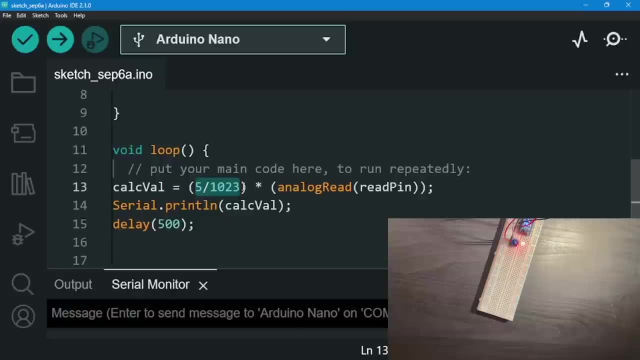 So the problem here is: let me just show you what I did. The problem here is what I'm using integers. So right here it's going to bring what Five divided by 1023 is going to give us, what It's going to give us a decimal. So what happens is it's going to what It's going to value? 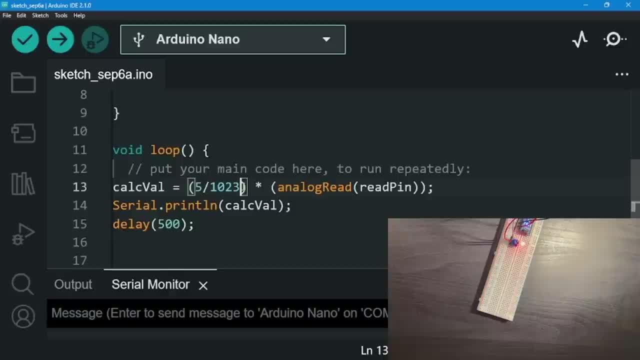 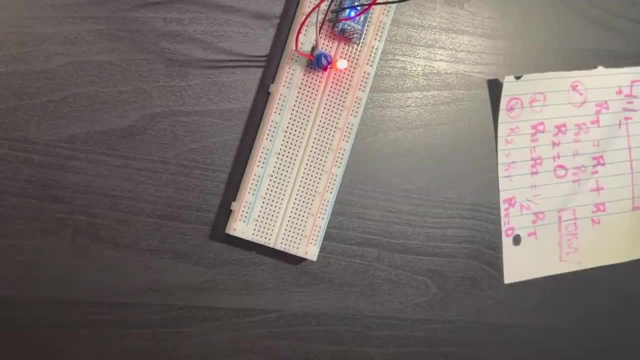 it's going to what It's going to? round it down to zero. Because if you just think of it, let me just divide five by 1023.. Let me just divide five by 1023.. Let me just bring my calculator right here. Let me just bring my calculator right here. I'm just turning out. 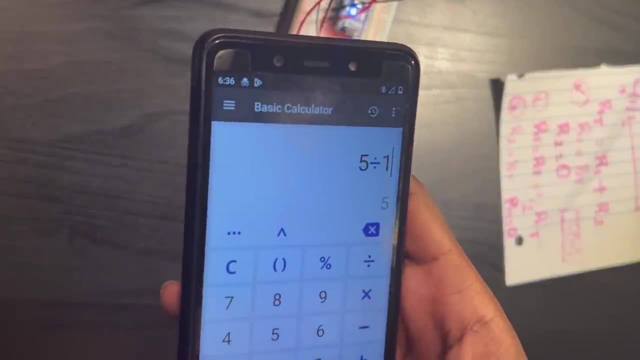 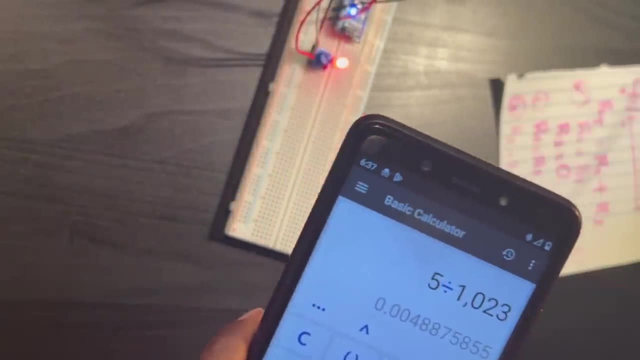 my calculator. Let me just divide five: 10, 23.. 10, 23.. It's almost what. It's almost zero And it's what It's rounding it. It's rounding it to what? It's rounding it to zero. So any number multiplied by zero coming from the analog, it's. 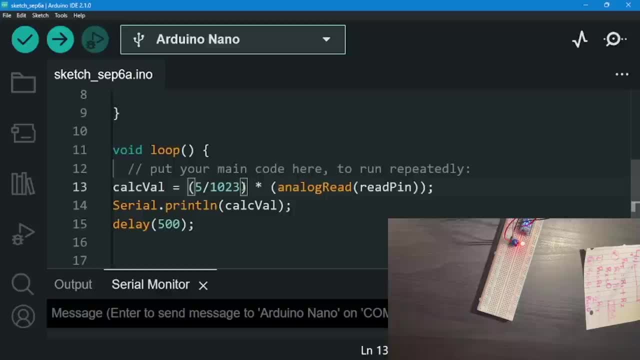 going to always read what It's going to always read: zero. So what do we need to do? We need to set it as what? As? decimals. So I go right here and what I'm going to do is set a point next to. 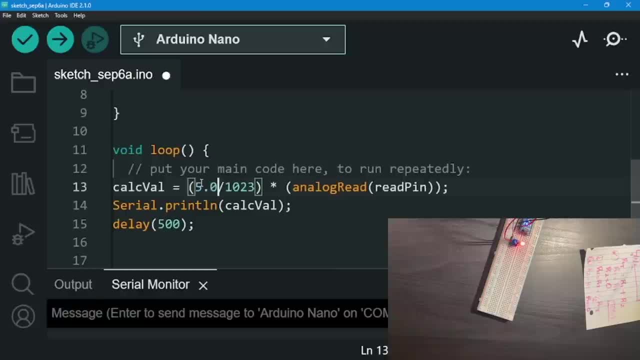 it All right. So I'm going to set a point next to it and you can see 5.0, or just the point next to it. It doesn't really matter, It's up to you. So I'm going to set a point next to it. And one final. 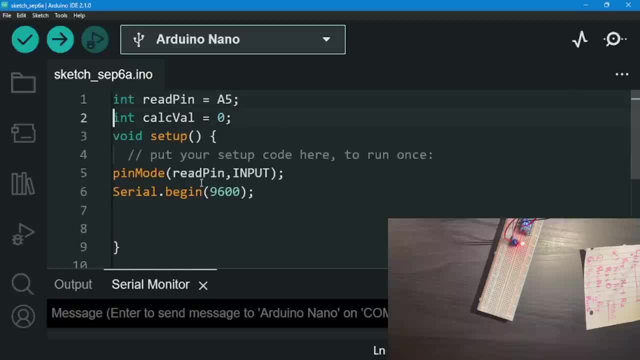 thing I need to do is what I need: to go to CalcVal right here, and I'm not going to set it to integers. I'm going to set it to float. Basically, float means what? Basically float means decimals. All right, So you can just set it up without actually giving it a value. It's up to you. 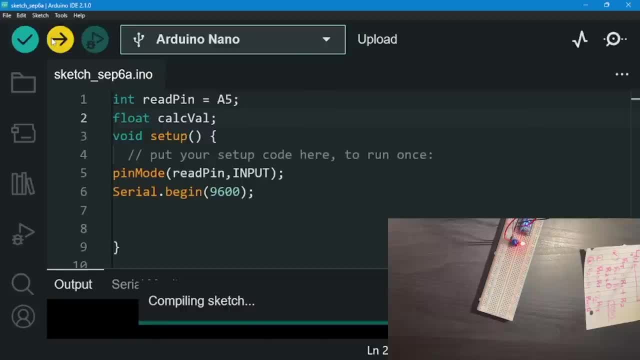 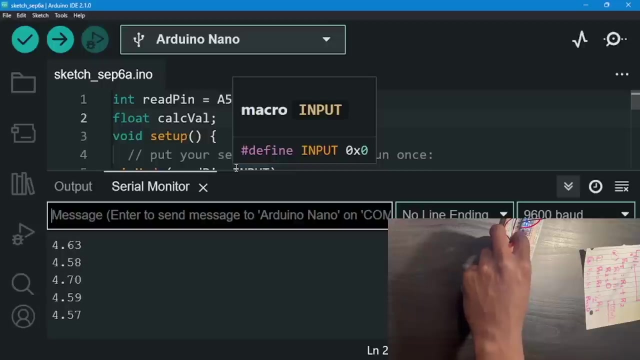 Let me just upload it right now. Okay, And it should be working. Okay, Stem compiling, Stem compiling. Okay, It should be done uploading by now. Let me open my serial monitor right here. All right, We're starting to receive real numbers here. Okay, We're receiving 4.7, 4.5 right here. 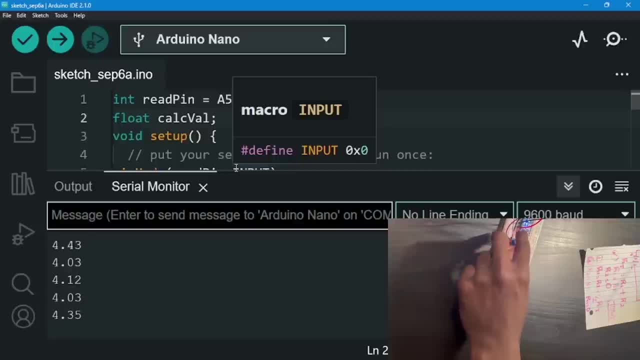 4.2.. We're not receiving full 5 volts. You know you might be wondering why. If I remove this LED right now, we're almost going to receive 5 volts. You see that As soon as I remove the LED. 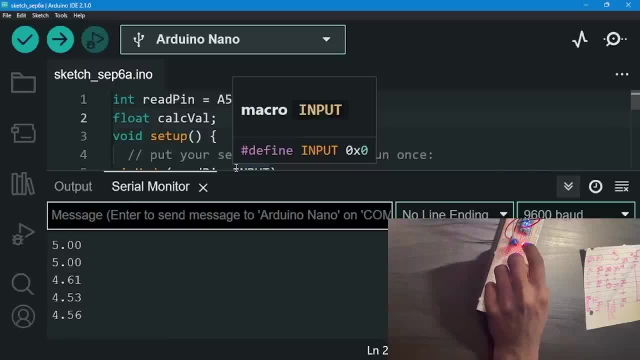 we get 5 volts because our LED is what. Our LED is using up some of the voltage right here. That's what? Okay, So it's using some of the The, what, The voltage. If I remove it right now, if I remove this LED right now, it's going to be. 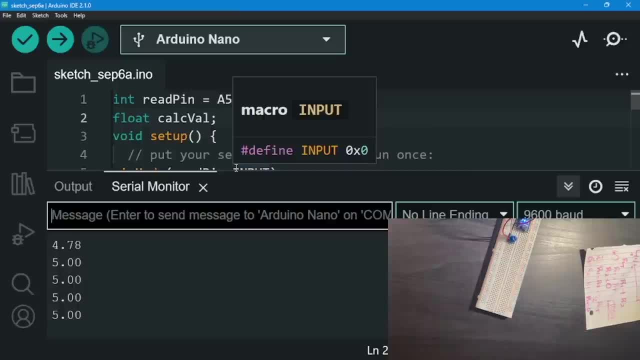 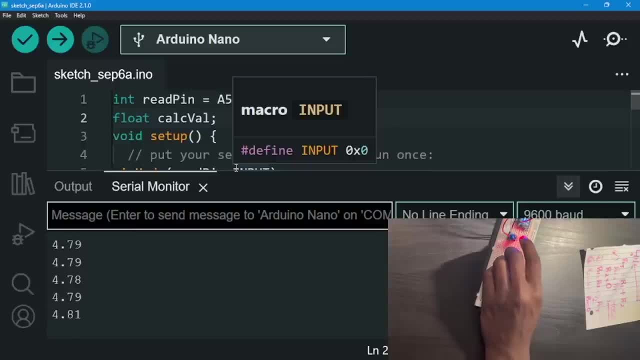 it back in, it's going to be giving me 4.8, because what It's going to be using 0, what 0.2 volt? right here, Our LED is using what 2.0.2 volt of the value? Okay, So let's just adjust it again, just. 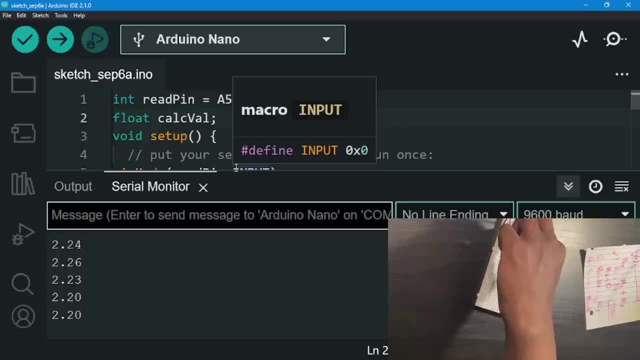 to check it out. Adjust it, Adjust it more, Adjust it Again, adjust it almost off right now, And there you have it, And that's it for this project. So I think we built something with a potentiometer. I think it's one of this higher. 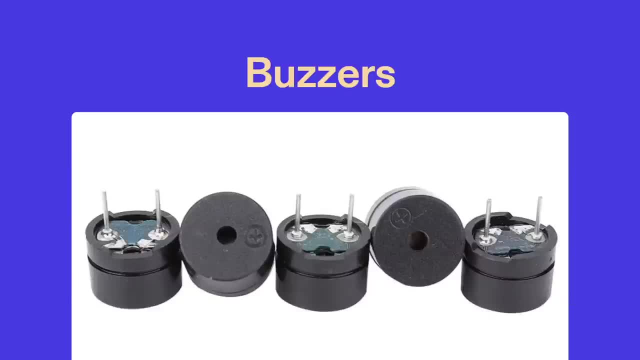 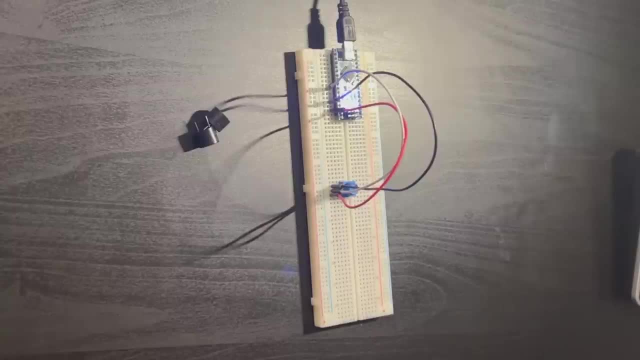 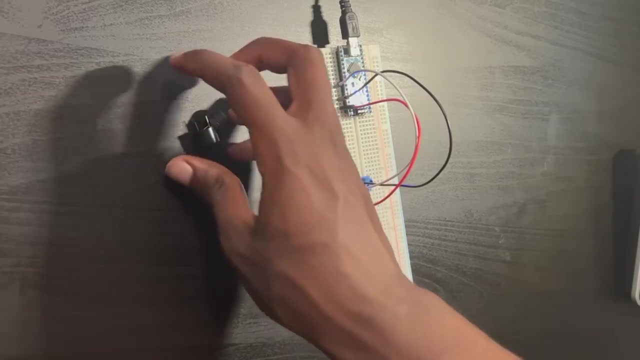 end of projects that are actually nice, So okay, So I did not change my circuit here. It's the same from the previous one, but we're going to add something. We're going to add something called buzzers. So if you look closely right now, let me just bring it. 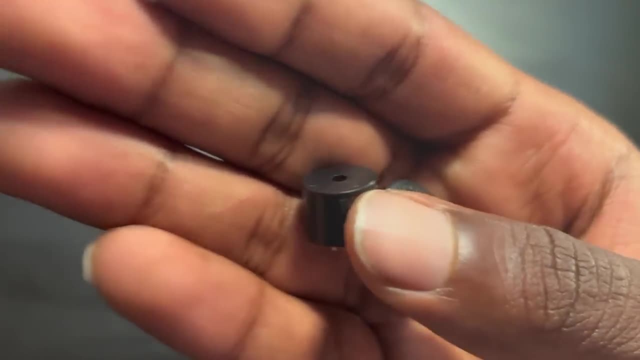 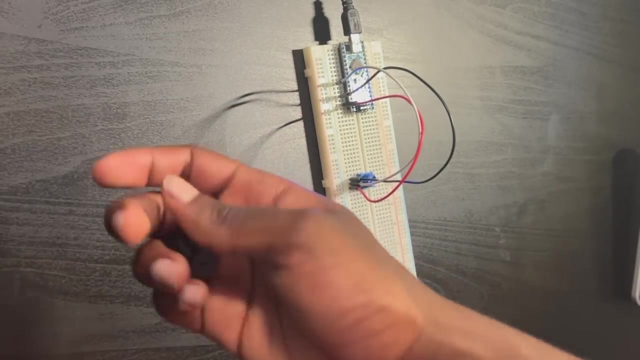 close enough. These are called buzzers and we're going to use them to basically create sound. So we're just going to change elliptical energy to what, To sound energy, basically by what? By vibrating. So again, before working with these buzzers, let's go in depth and try to understand. 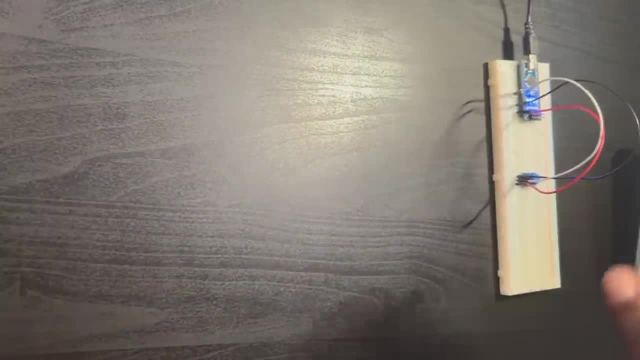 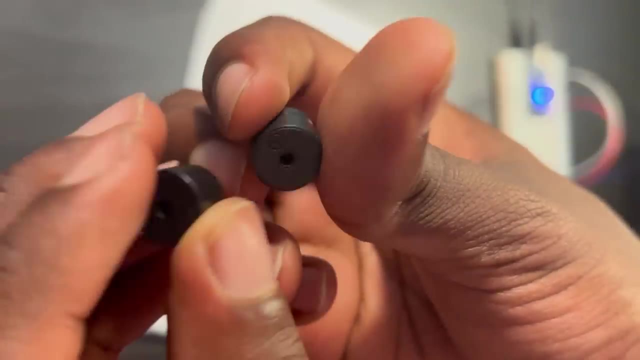 what they do. So let's just have a rough idea of what buzzers are. Okay, So if you look close enough, again, these are called buzzers. If you look close enough, you can see that they're not the same thing. If you look at top they might seem like they're the same thing, but if you look 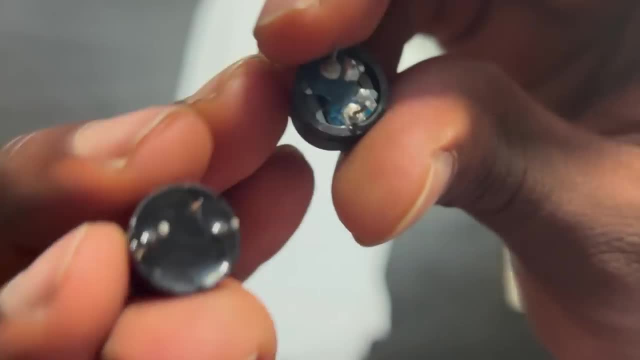 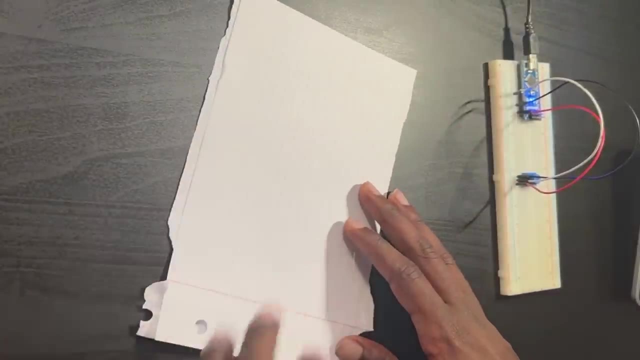 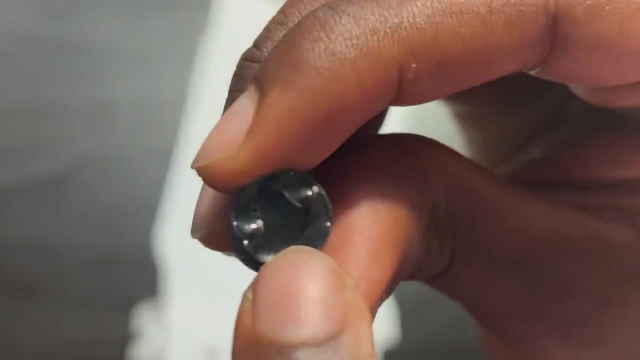 at the bottom. there's a black one right here, Okay, And there's a one where you can see the circuit, Okay. So let's just go here and try to understand what they are. So the one marked with a black one is a what is called an active buzzer. Okay, An active buzzer, And the one that does not. 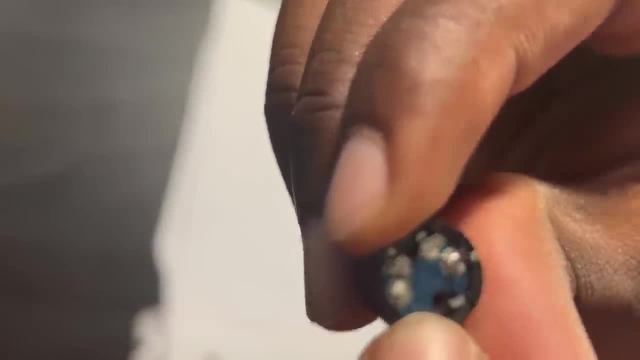 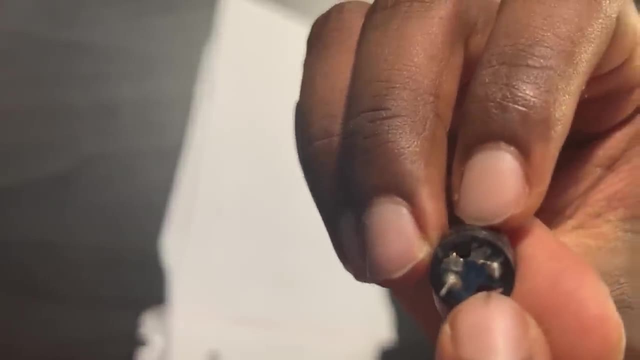 have any board, any uh on it where you can see the uh, where you can see the components. right here is what is called a passive buzzer. Okay, So I want you to understand the difference between these two. So both of them. 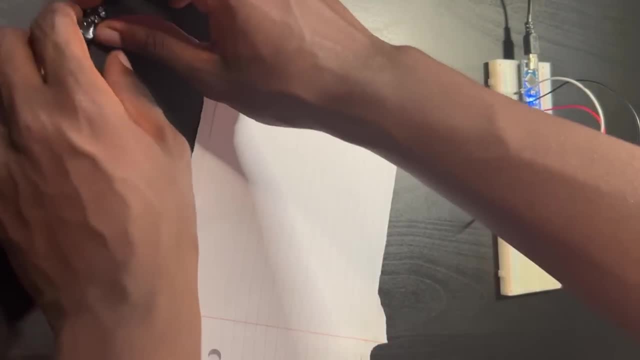 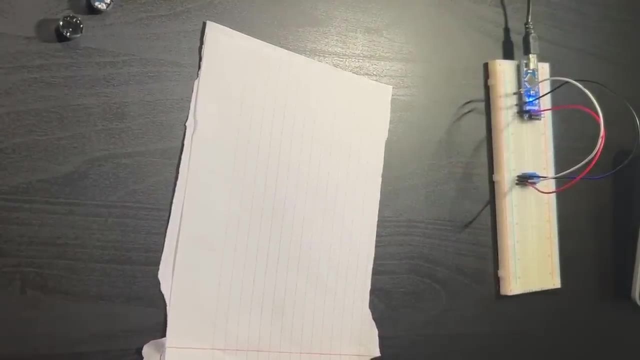 are used to create sounds, but it's going to be different for both of them. So let's go right here and let me just explain what an active buzzer is. Okay, Just do that. So an active buzzer: what it basically does is what. 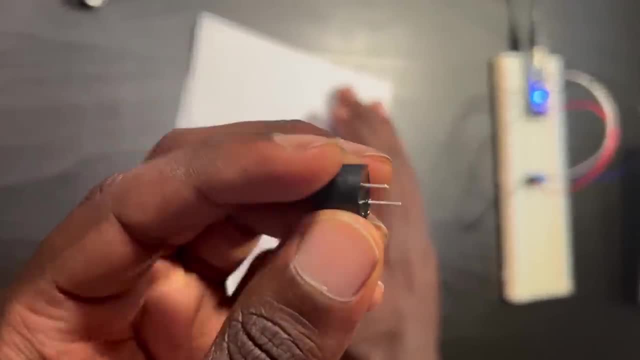 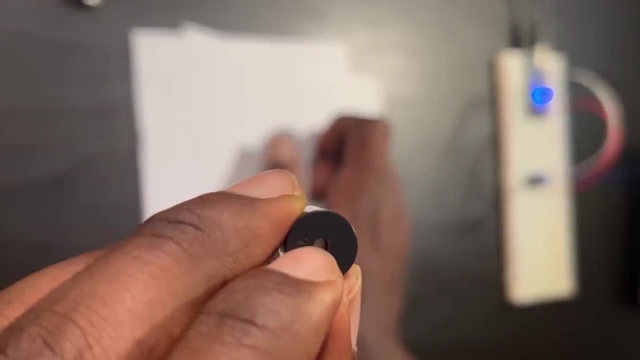 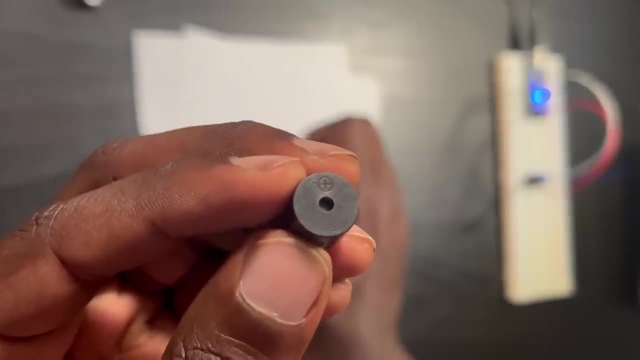 It needs DC voltage, It takes DC voltage And what basically happens is there. if you look inside, if you just pry it up open, there's a cone that vibrates- Okay. There's a cone that vibrates back and forth, back and forth- Okay, There's a cone that what that vibrates back and forth and 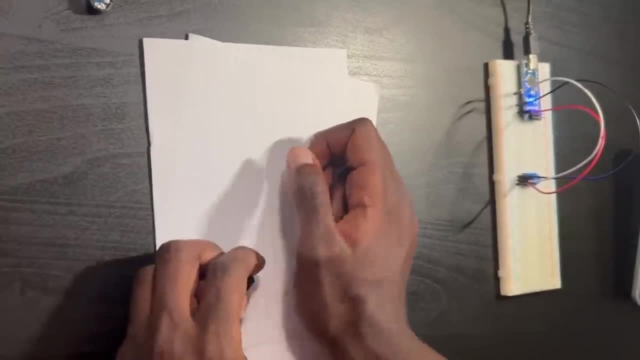 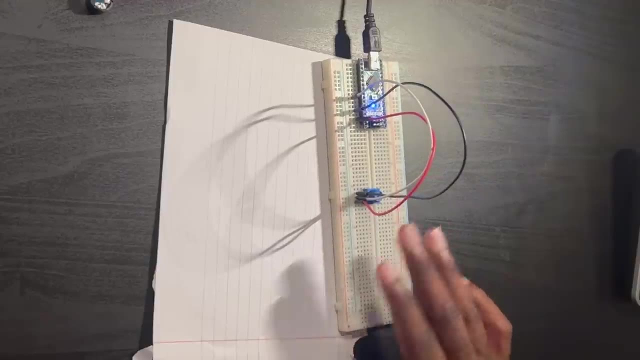 basically what creates sound by vibration. So let's just do that. So I have my again circuit from the previous lesson. So what I'm going to do is I'm not going to touch this one. I'm not going to touch any of these, I'm just going to. 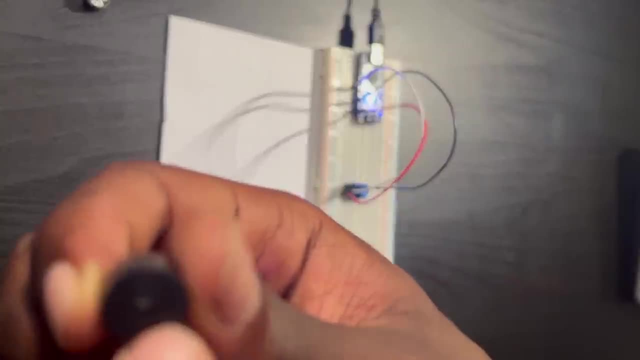 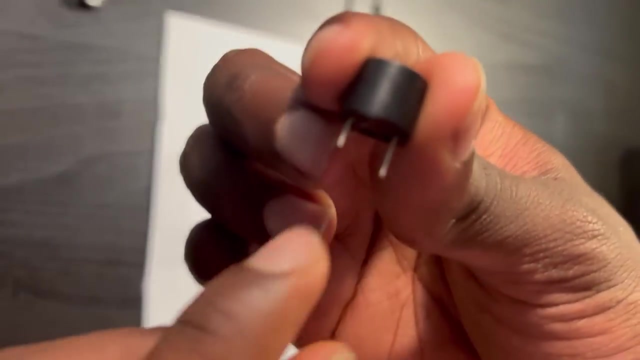 give it a new space. And one important thing you need to understand is these things: if you look at it, it has a plus sign Okay. So not only that too, but even there's a difference in what. There's a difference in their what, In the length. Can you see that this one is longer? 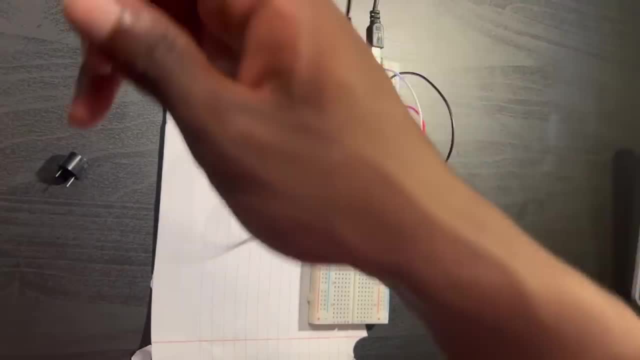 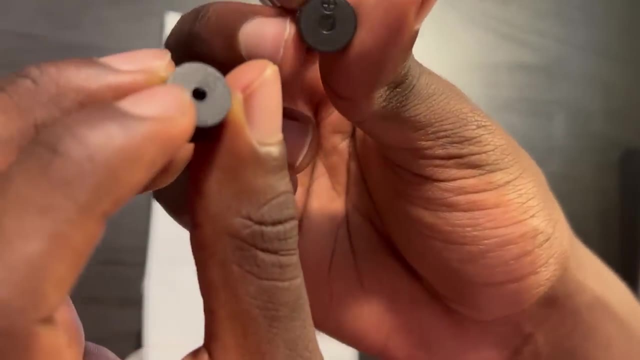 The plus sign is what Is longer. Just like what. Just like when we were using what LEDs. So keep that in mind. both of them have what. Both of them have a plus side, both of them have a plus sign and the plus sign: what Leg is longer? Okay, Okay, Then I'm going to go ahead and do this. So let's do that. So you did that. You want to start with the long one and then you're going to add in the long one. So the long one is: you're going to add in the long one, This one, right here. 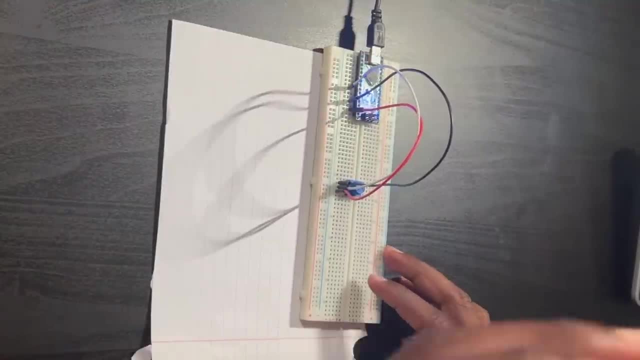 longer. okay, so let's go back to our active buzzer right here. all i need to do is put the plus sign around here and what i'm going to do is connect it to the five volt. so let me just go to five volt. right here there's the five volt and i'm just going to connect to the longer side of it. 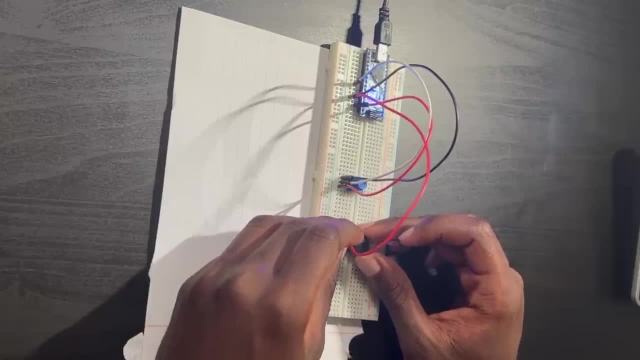 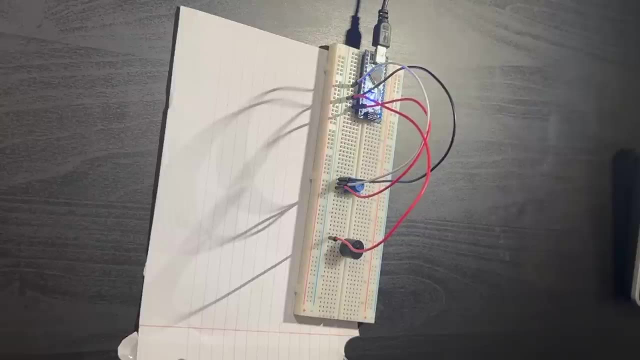 or basically the positive side. that's all i'm going to do, okay, and let me bring another wire right here. let's get another wire. i'm sure this is a very short wire. let me get a longer wire. let me get a longer wire right here. all of them are short today. i have to go closer, if not. 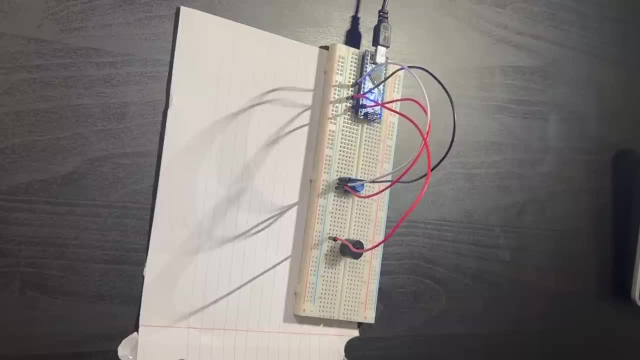 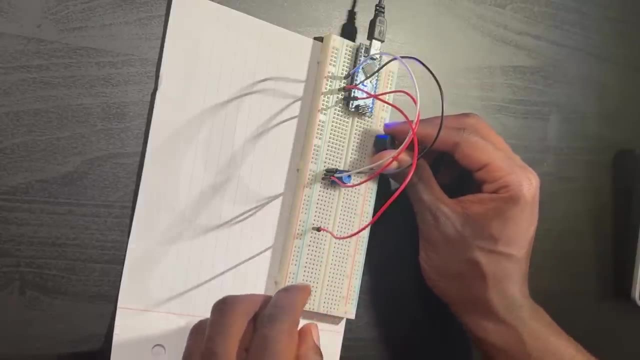 all of them are short. i don't have any longer wires left. i've used all of my longer wires, okay, so if i have a short one, what i'm gonna do is go through this side. let me just go back to this side, okay, and let me just take this five volt right here and take it. 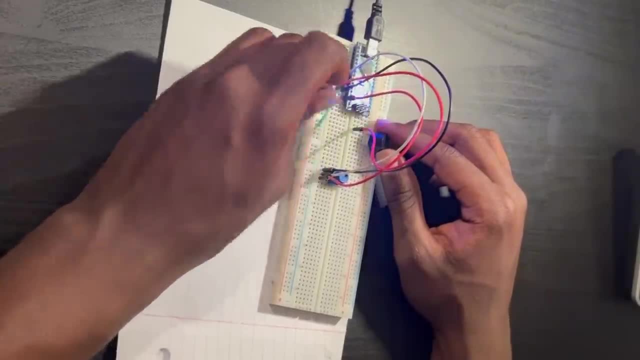 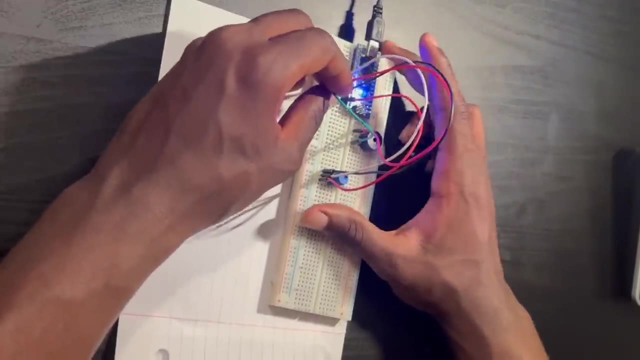 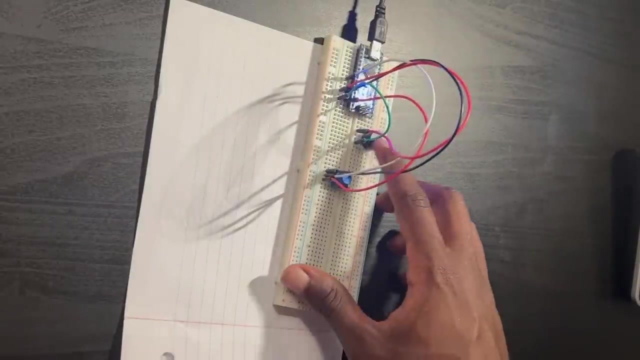 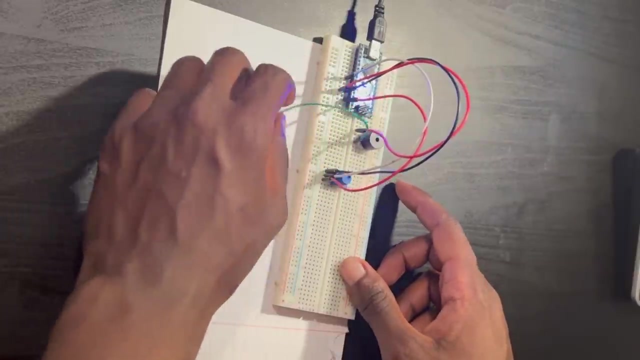 okay and put it right here. i've got the gnd, the ground pin. this is gonna- i'm gonna connect the negative side to what, the gnd? so let me just do that. that's the gnd right here and it starts to make what can you hear? that starts to make what sound directly as i plug it in. so, okay, that's what. 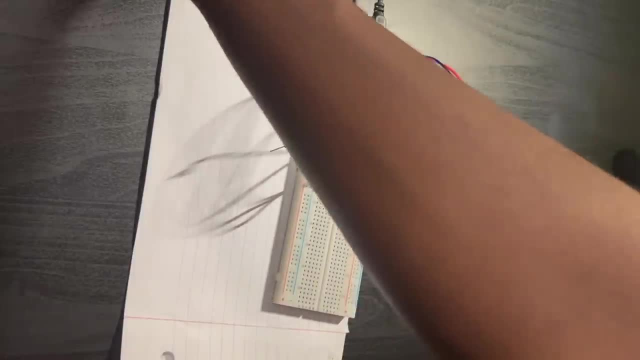 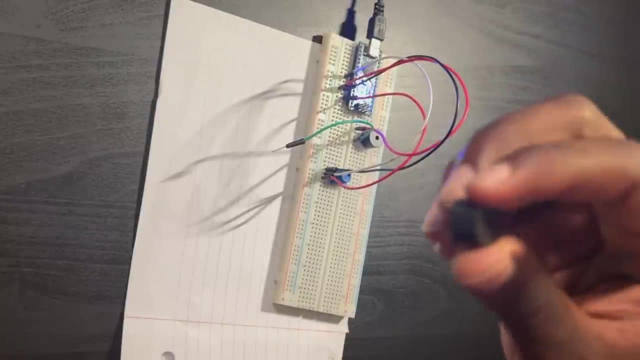 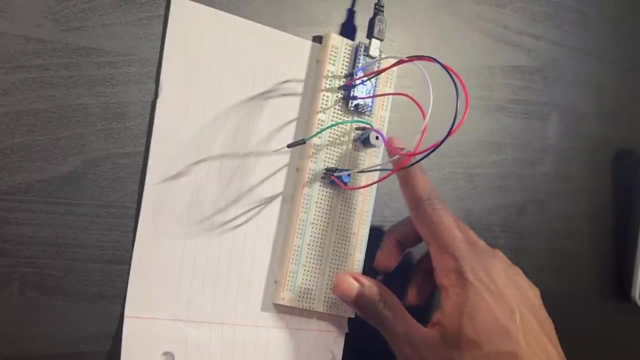 a, an, an. an active buzzer does okay, so let me just bring this one, the passive buzzer. okay. when i'm using a passive buzzer, one thing that's necessary to do is what the difference that comes here is. i need to use ac. basically, i need to use what ac circuit for this one. i've just directly used what five volt. 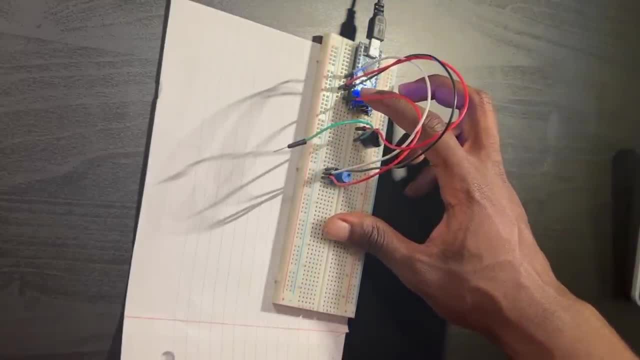 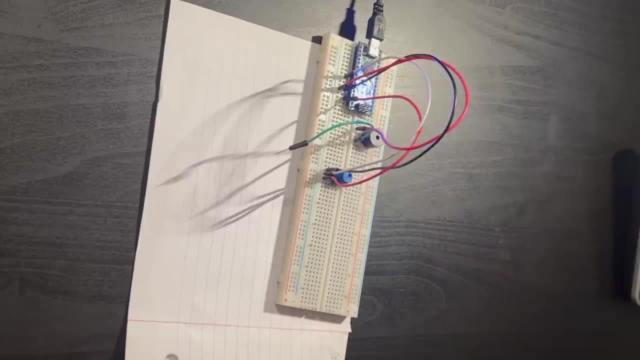 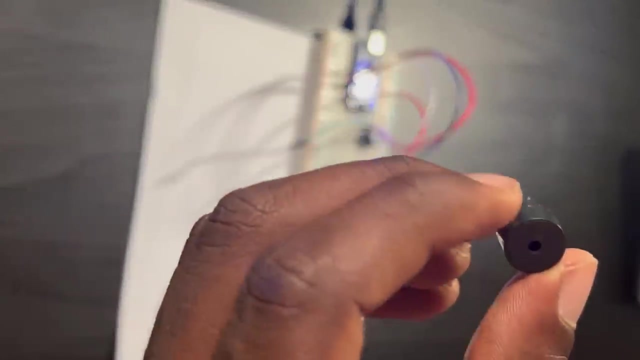 when you look at the arduino, uh, five volt, right here, the five volt pin, it directly outputs five volt dc. basically, what direct current? i'm gonna come back to this and actually compare and contrast them, but i use what direct current? okay, so for this one we're gonna use ac current. 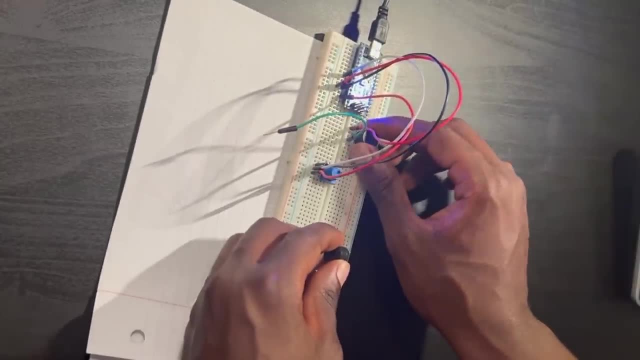 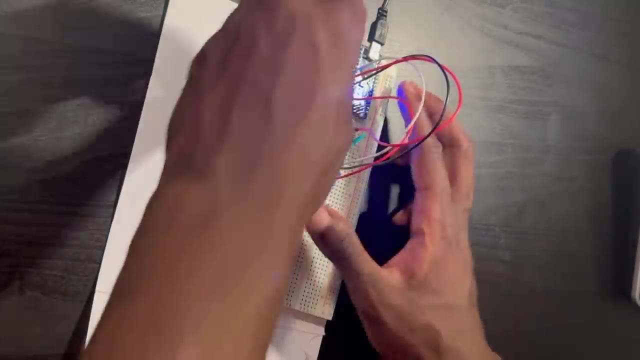 alternative current. okay, so let me just uh remove my uh active buzzer here. this is my active buzzer again, the one with the black one. let me just remove it. let me just remove the wires that i used for the active buzzer so that it does not get too messy. let's do that. 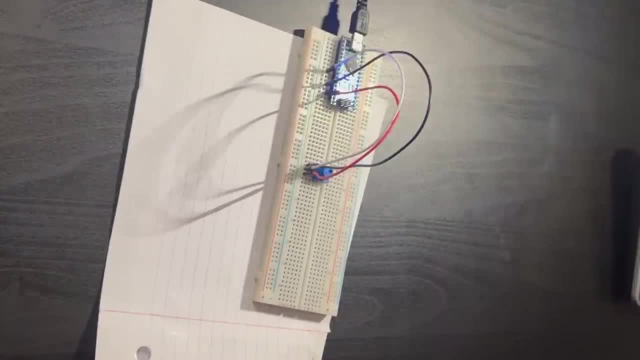 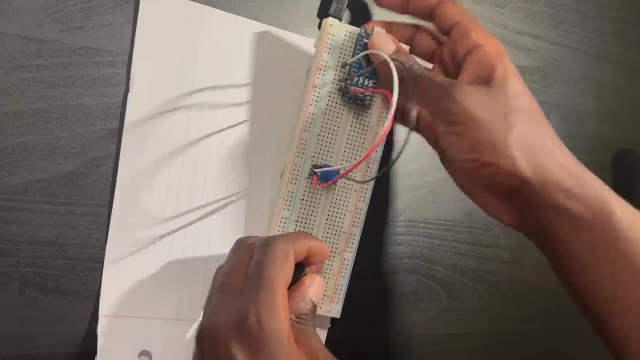 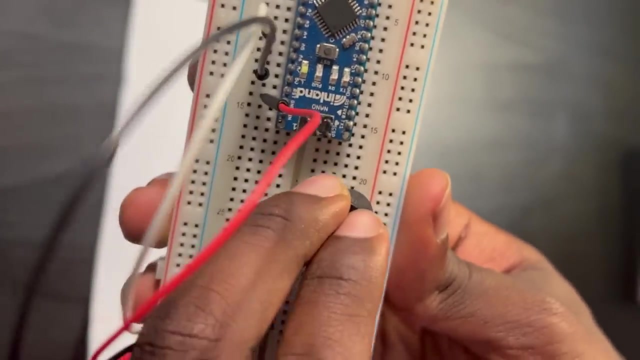 okay, and now i'm gonna do right here i have again my uh passive buzzer. let me just set it up. let me just unplug my arduino now. let me just go back closer so you can actually see it. there's my uh passables. i'm just going to put it right there. same spot. actually, i need to need my gnd pin. 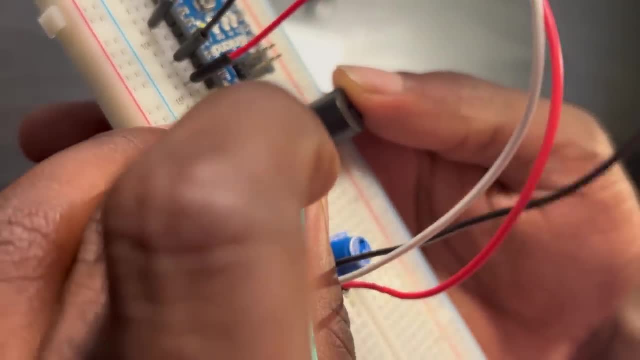 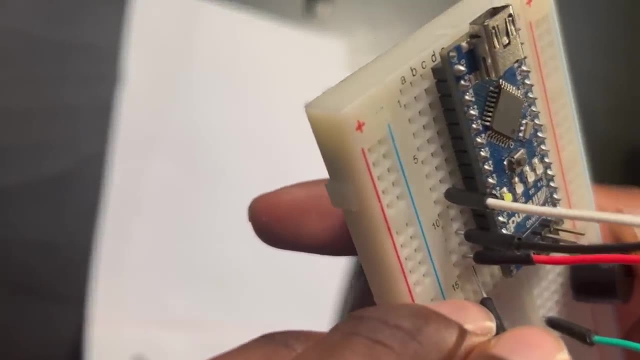 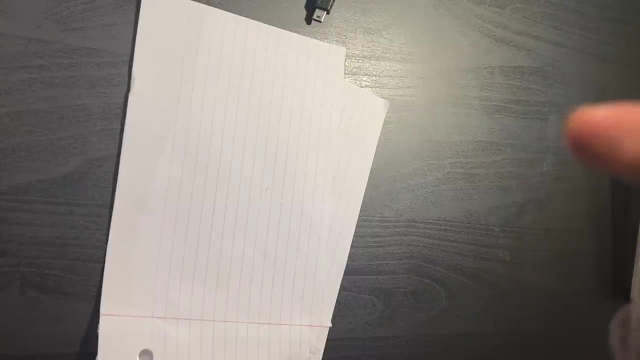 connected to here. my gnd can't see it. all right, there we go: gnd pin connected to the negative side from the other leg, which is connected here, and the positive side. i'm going to be using what? those digital pins that are marked with a what, with a squiggly sign. 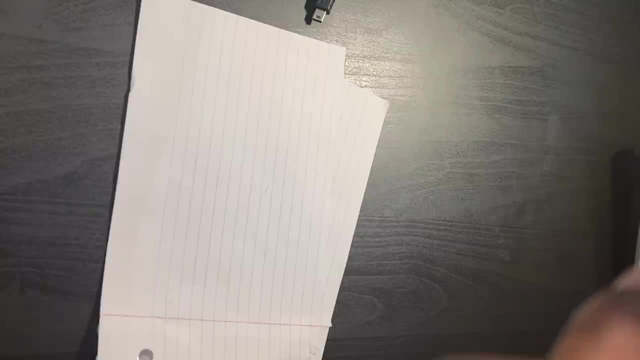 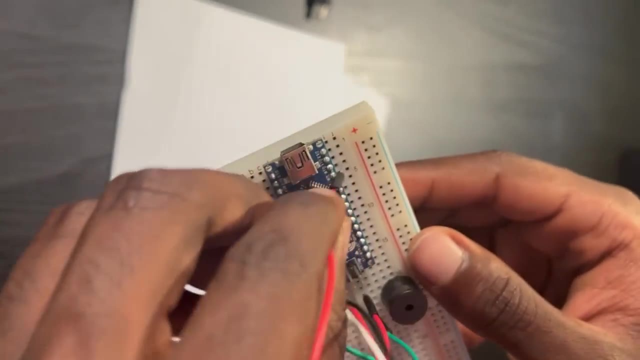 those ones that i said that are that behave both as a digital pin and also as a what it's, an analog pin. okay, so we're going to work with those. let me just put a digital pin 9. okay, digital pin 9 because of what it has. what? if you look closely again, it has what it has: a dot sign. 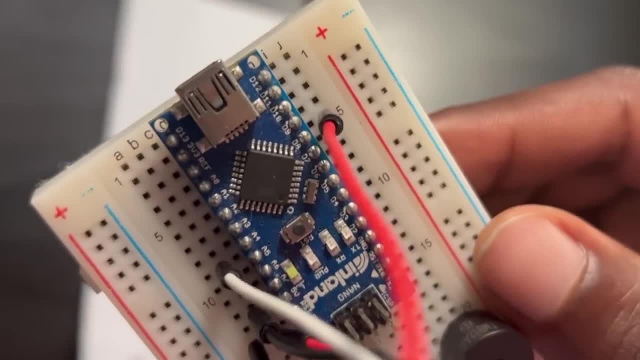 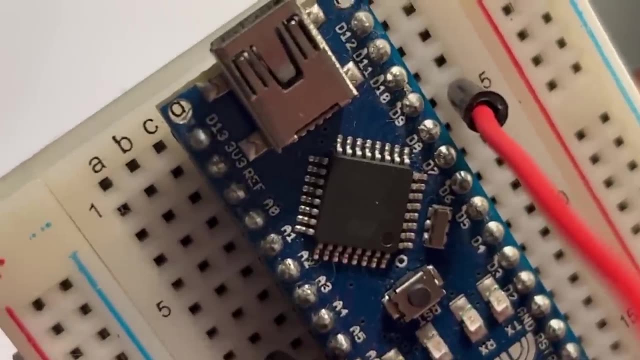 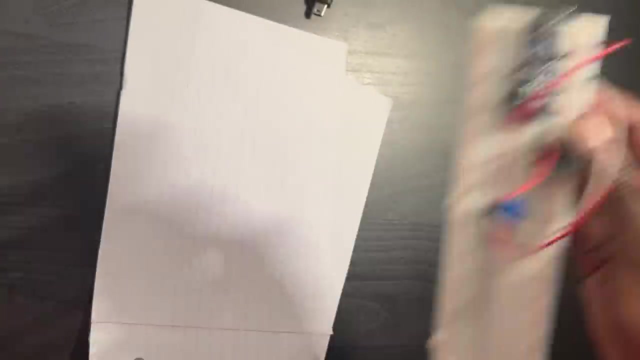 let me just bring it close enough so that it focuses. let me just actually zoom in more. you see that it has a dot sign right there, so we're going to use those pins again that i mentioned that, the ones that i used for what? for analog, right right now, let me just zoom out. okay, zoom it out. 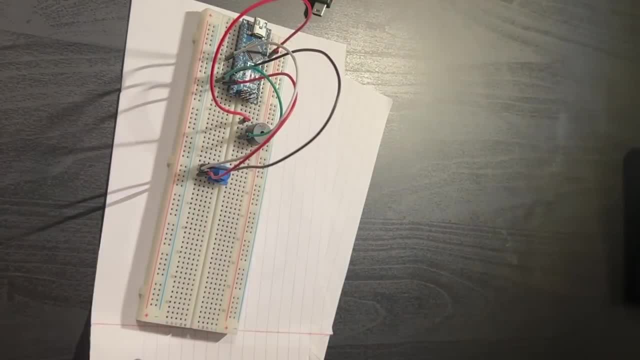 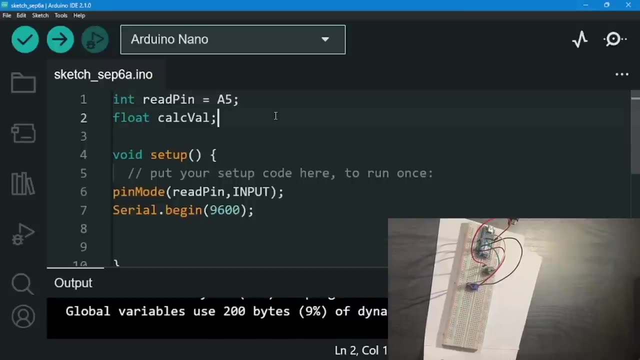 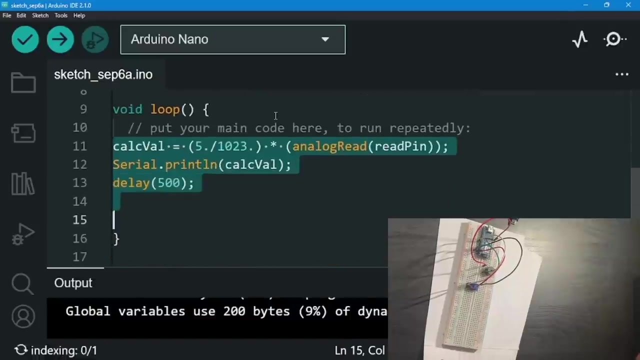 okay, so that's what i'm gonna do. so let me go over to my screen right now and then actually write down some code. so let me just, uh, remove this from here now, move this code, if that would be good. right now we can write it down if you need to again. 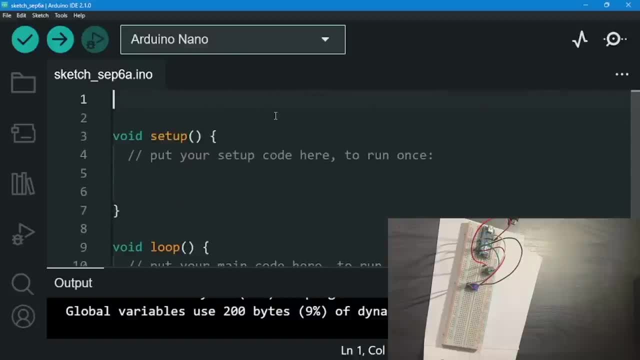 okay. so what i'm going to do is what we're going to need- additional pins. i'm going to say, is what i'm going to need, that there's still pin 9. so i'm going to say what? what is this passive buzz? it's going to say passive buzz. it's going to be what i'm going to say: that there's still pin 9. 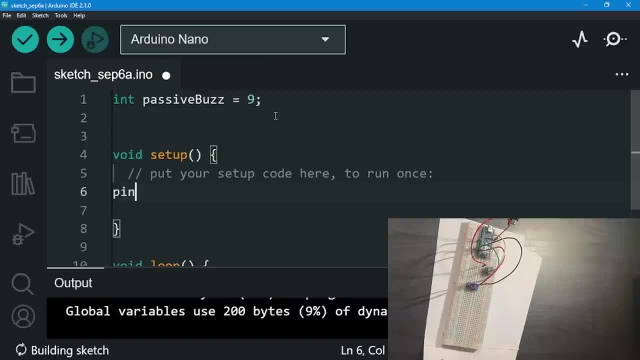 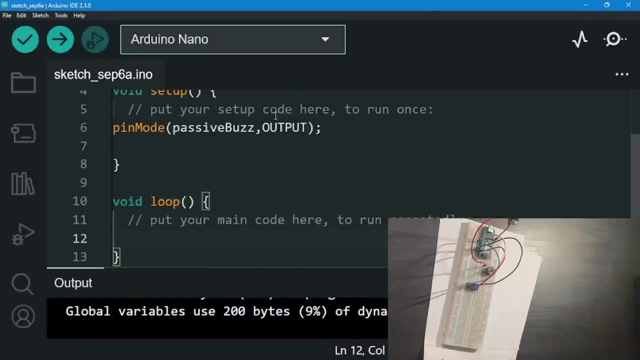 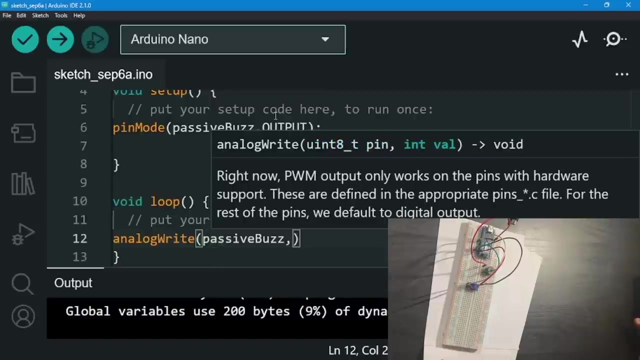 okay, well, i need to just watch or set it up. i'm going to say pass, it was. set it to what as an output? there you go then afterwards, what i need to do, i'm going to need to do is what? use the analog write command and again use passive, again buzz, and then what? then let me just set it to. 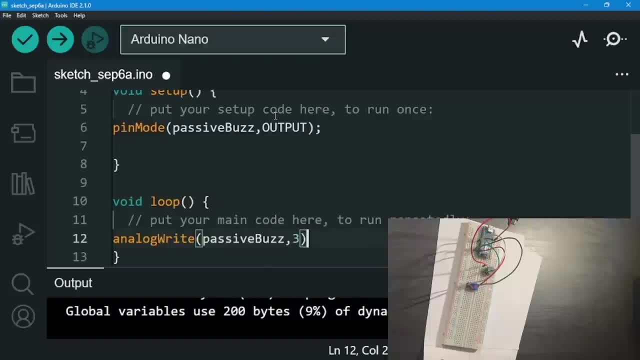 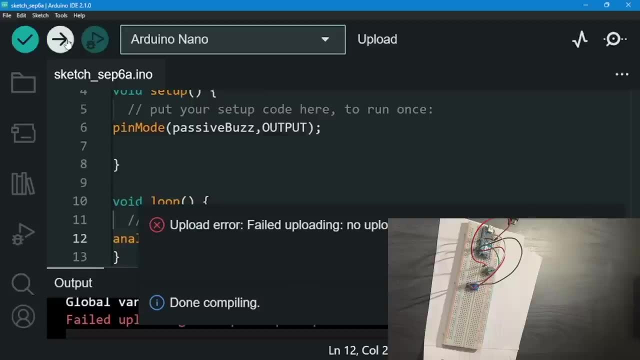 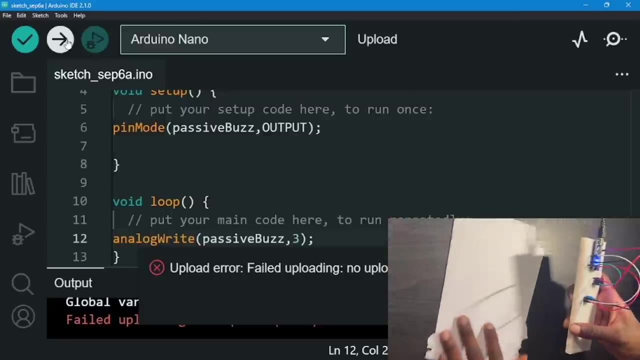 whatever i want to. let's just say i want to set it to three. okay, so let me just it three. let me just upload this right now. it's done compiling. we cannot upload it because what we have not plugged, our arduino. let me just do that right here. let me just do that, let me show. 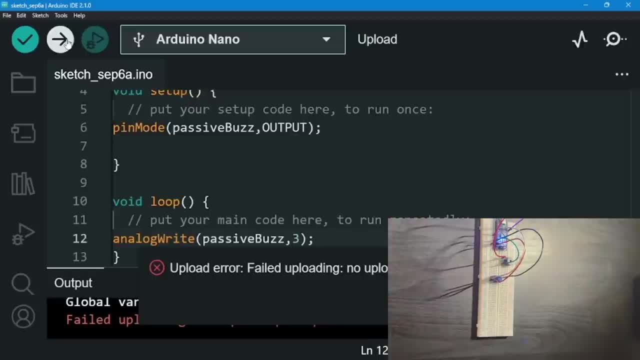 up the paper. for now, i'm gonna go with the explanation after we work with it a bit. okay, let's just upload it. it's done compiling. okay, it's not uploading. well, we can't hear anything, can we? i cannot hear anything. is everything all right? let me just again check my 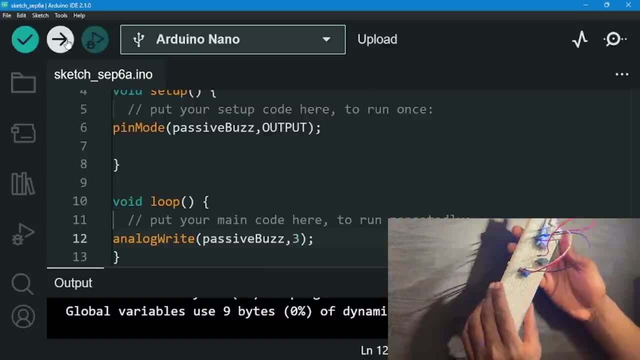 pins. okay, there's still a pin down this year. there we go. let me just stop it first. let me just stop it for a second. uh, you might not hear it as very, uh, you might not hear it as strong as the active buzzer, because i set it to what i set it to three. 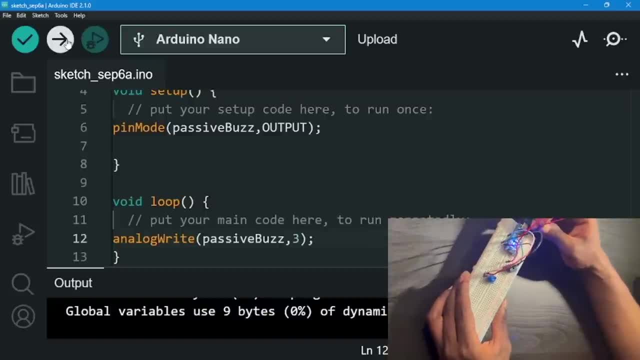 because it's going to be receiving less. what less electricity. it's going to be receiving less current. okay, let's do that again. hopefully you can hear it. if not, let me just again increase the value here. just put three. so let's just increase it to: uh, let's just say 20 for now. just say 20.. 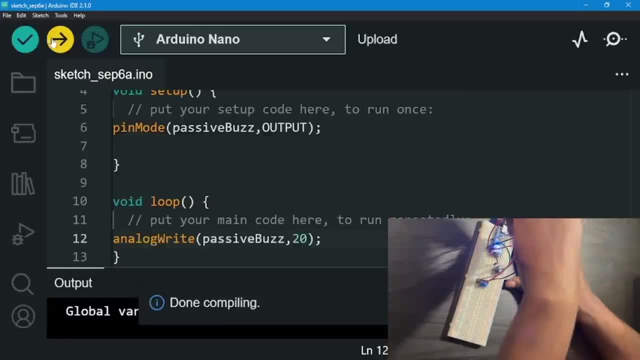 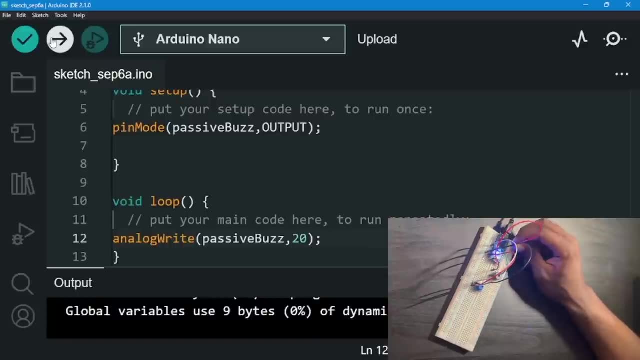 let me just again put back what they're still pin nine back again to its spot. now it's louder. now it's louder. okay, let's raise it to a higher value. let's just say 40 or 50.. we set it to 50.. 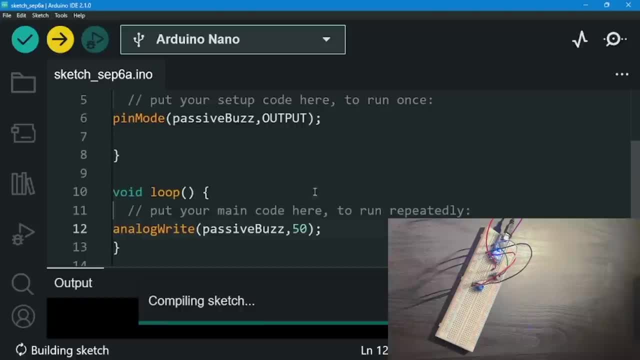 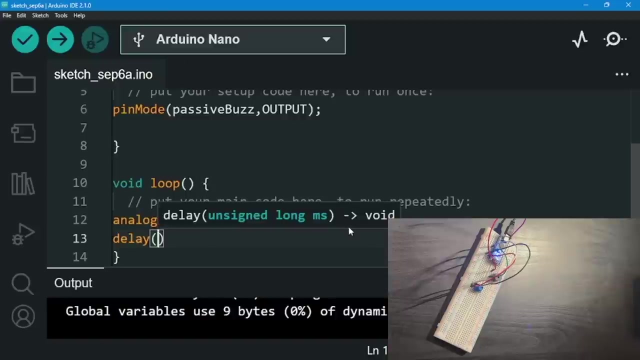 let's upload it right now. it's done compiling. it's done uploading. let me put it back right here, now we can hear it louder, all right, so let's make it actually do. something interesting is, we do is put a delay on it, all right, so we're just going to set it on and off, on and on, on and off, because it's going to sound. 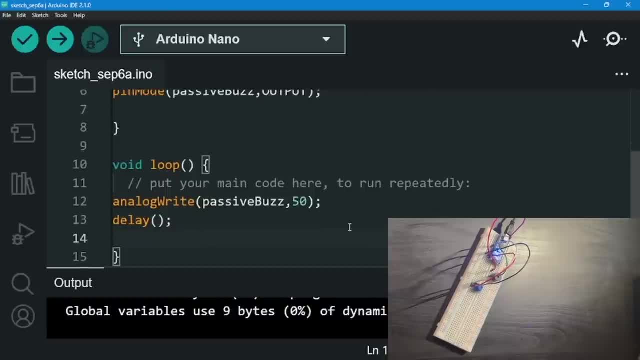 better that way. so let me see delay right here and i'll log right what passive buzz to set it to zero right here and give it a delay again, okay, so one thing i did not do right here is set up what, how much i want to set it to be. so let's. 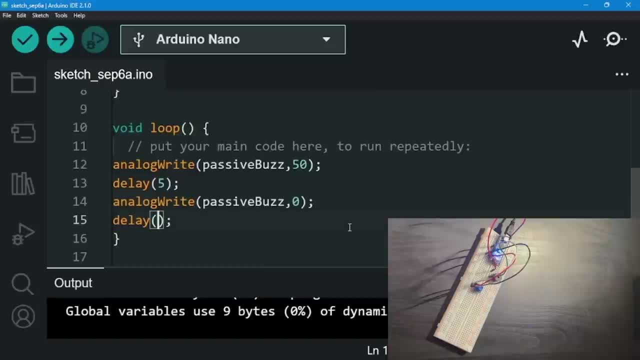 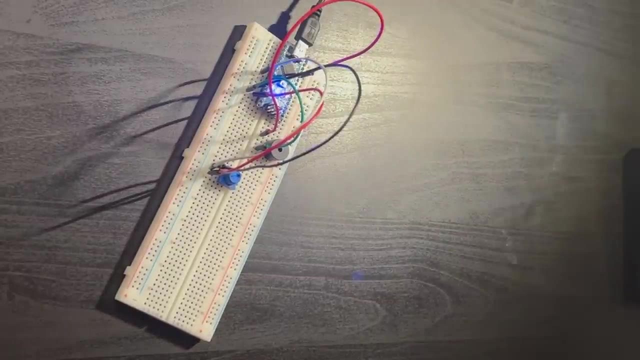 just say again five milliseconds. again i'm saying five milliseconds and let's upload it again. let me just put it back right here. the d button come here, all right, let's just set this, maybe to delay one. i need to delay, uh, about 10. let's just say: you want a longer delay. 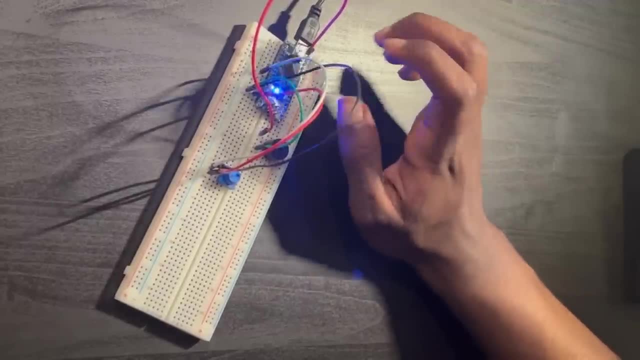 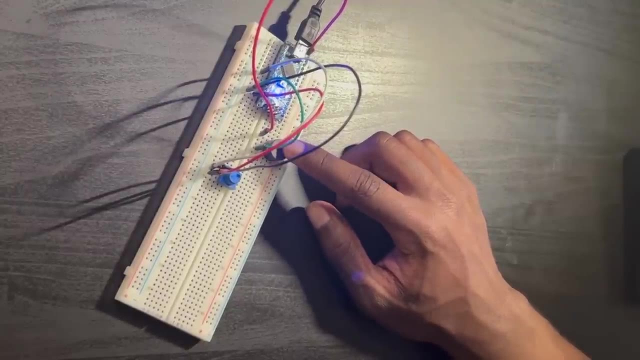 all right, we've experimented with the, the passive buzzer and the active buzzer, and one thing the passive buzzer you know is capable of is what you can turn it off and turn it on. can you do that? can you see that you can turn it on and off, as we did right here? we turn 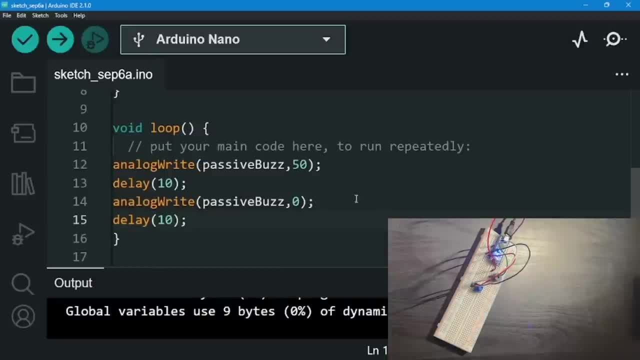 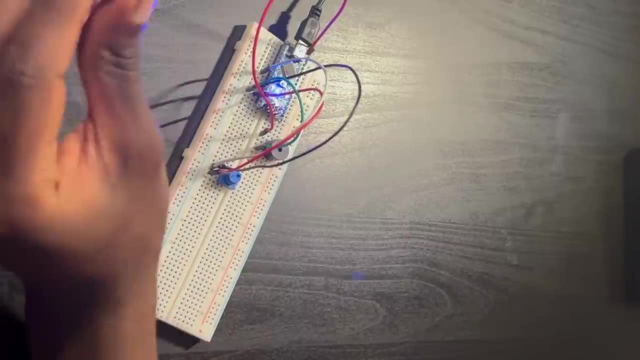 this to what? to zero, basically what? turning it off at line 14. you basically want turn off. we instead, as one turn off buzzer. that's what we did right here. what did we do? we turn on buzzer. well, we couldn't do that using what? using an active buzzer. why is that so? why is that so we? 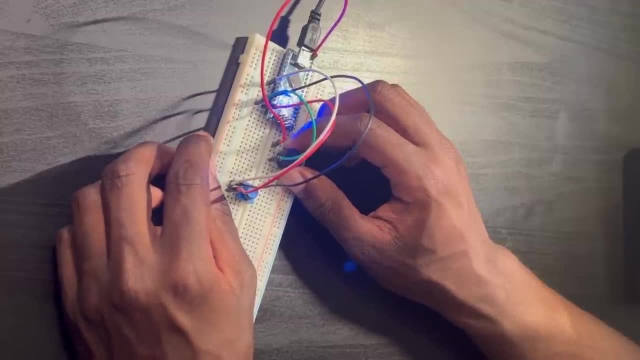 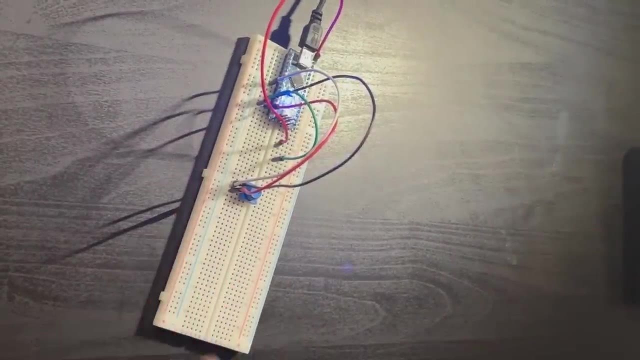 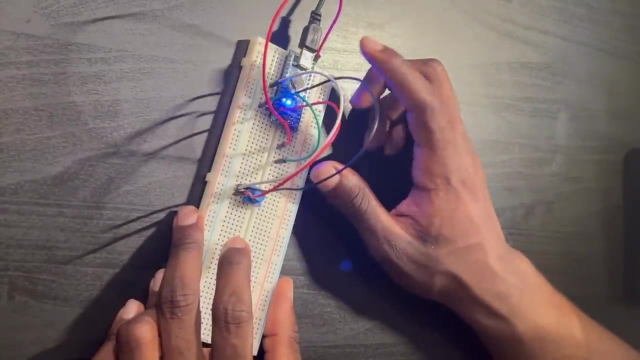 can't do that using an active buzzer. why is that so? so, um, the big thing here is: when using an active buzzer is what? why couldn't we do that? well, it's because what five volt is always what five volt. five volt always outputs what five volt. okay, so five volt, always apple, what outputs what five. 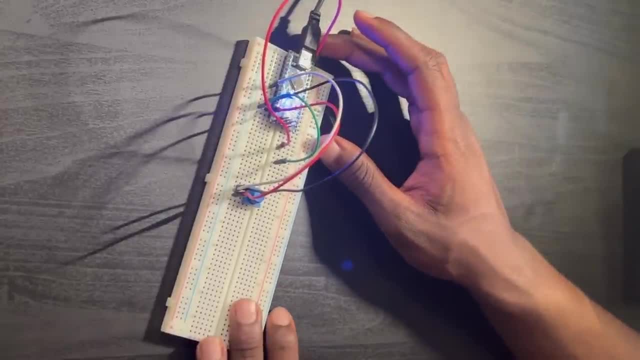 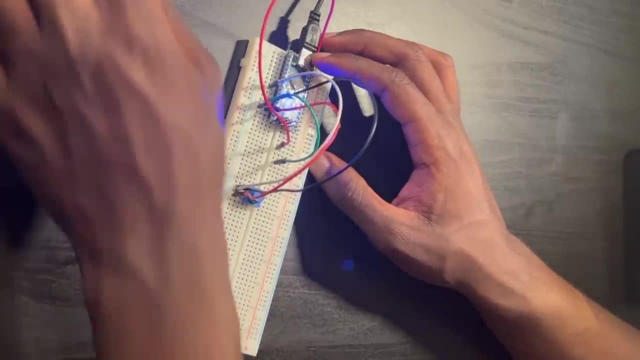 oh, that's why it cannot, you know, go on and off. that's why we cannot, you know, turn it on off, turned on off off. we cannot. we cannot do it using a five volt, but we can definitely do it using a digital pan, we can definitely do it using a distortion. um, okay, so with that in mind, 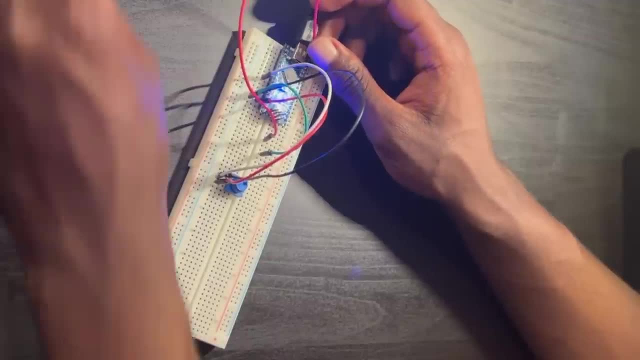 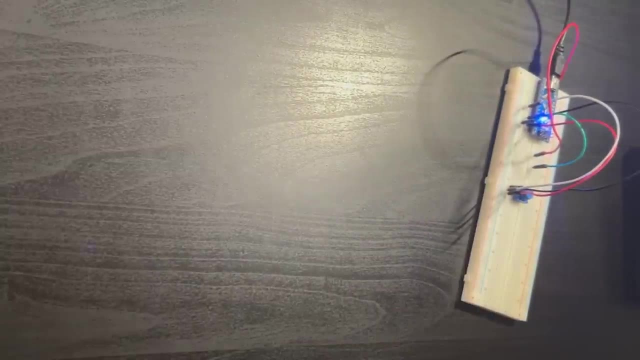 me just again, actually. so, with that in mind, actually what i'm going to do is going to be working with potential meters. before doing that, we're going to have to go again. what between? i have to go behind the sides here, so we're going to go to the sides. so let's do that, okay, so why? 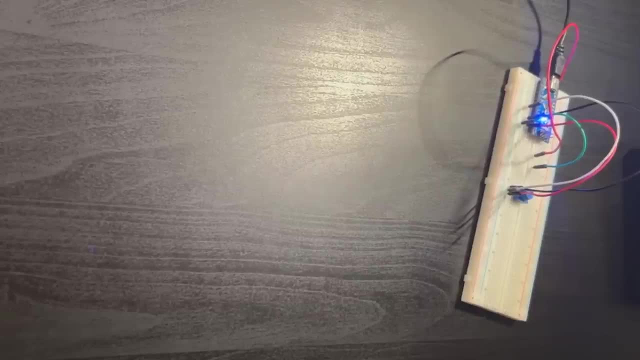 does a passive buzzer, you know, require ac circuit? why does a active buzzer require uh, why does an active buzzer require a dc circuit? a passive buzzer requires ac circuit and, uh, an active buzzer requires an, uh, a dc circuit. why is that so? why is that so so in a passive buzzer? okay, we use. 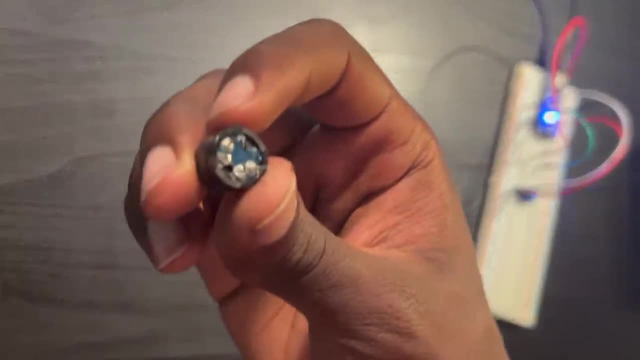 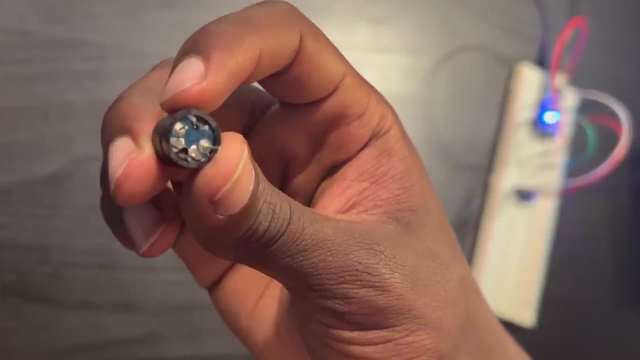 ac circuit. let me just bring a passive buzzer right here. we use ac circuit because what? because there's something called the vibration cone, a vibration cone. what it basically does is what it vibrates to create separate. okay, so the vibration cone one in the ac circuit, what? 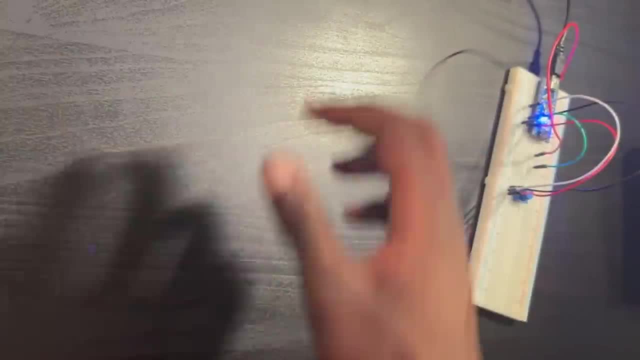 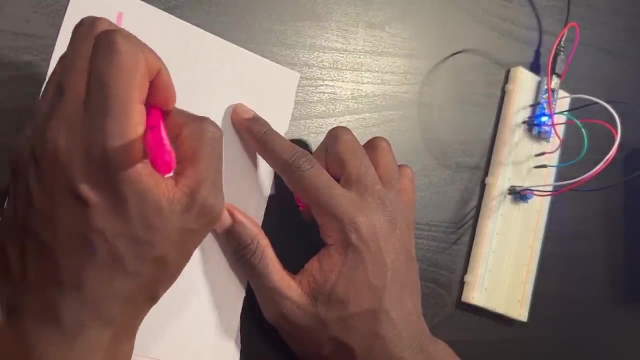 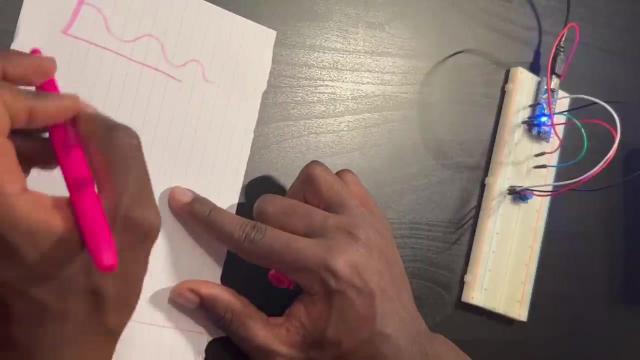 goes back and forth, back and forth. so one thing i want you to think of on the ac circuit is what. let's bring this right here. you've, i think most likely you've- heard the term easy circuit and you most likely know this graph. it goes up and down, up and down. when you look at a dc circuit, it's what it's. 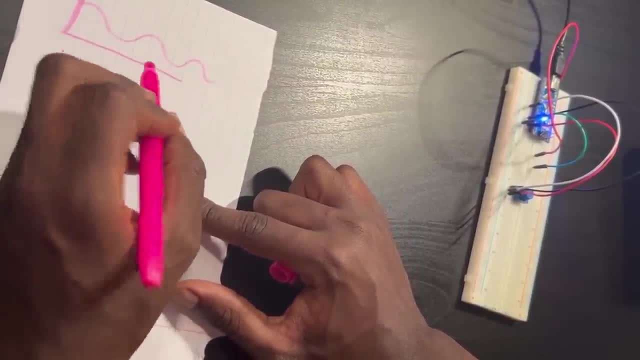 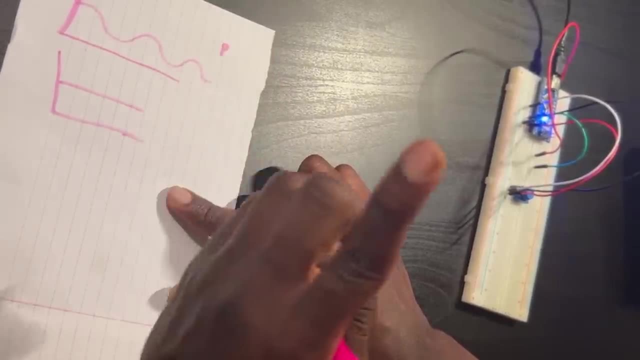 straight. it goes what. it goes one way. this goes what. this goes back and forth. this goes back and forth. basically what? basically vibrating? just think of it back and forth, back and forth. a very fine description of what it vibrates to basically, what can be vibrating when it vibrates, what? 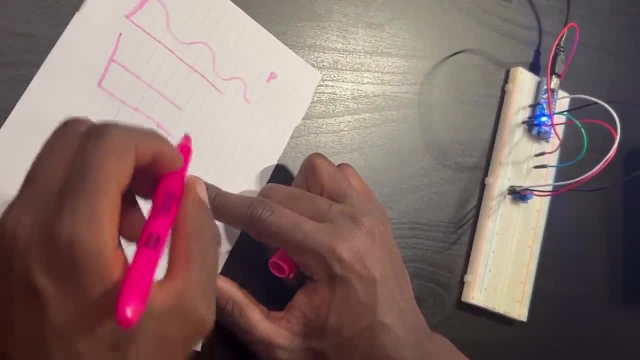 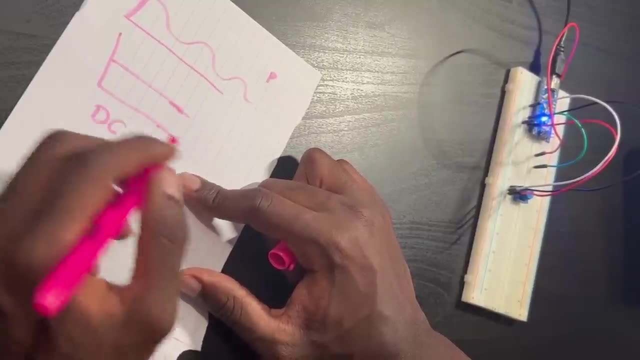 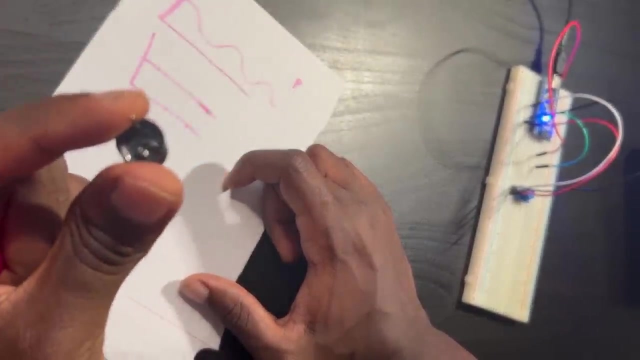 happens is that when it vibrates, it creates sound. okay, so when you think of, um, uh, uh, direct circuit right here, a dc circuit right here, you might be wondering then, how does uh, how does an active buzzer work then? because it receives what it receives. an active buzzer receives what an active. 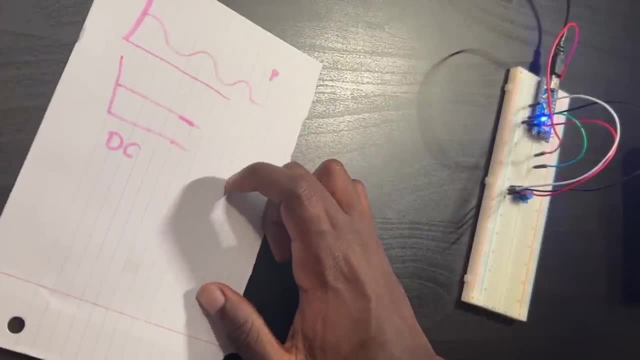 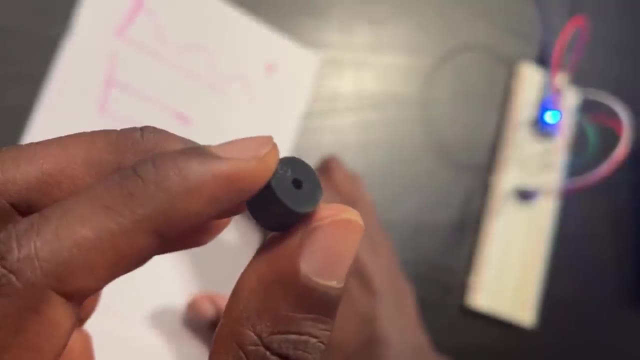 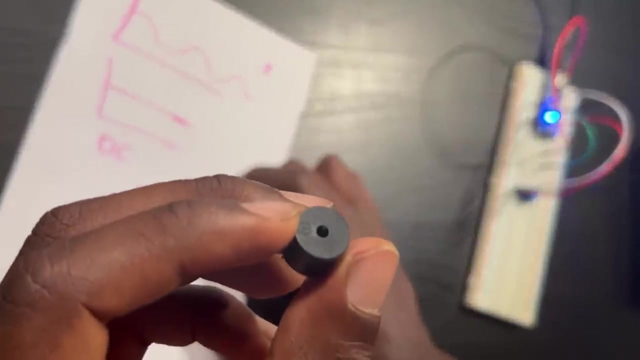 buzzer receives dc circuit. so when it comes towards this circuit, what happens is, when it comes to an active buzzer, what happens is the difference in component here is that it uses something called electromagnetic- electromagnetic, all right spectrum. so what it uses is what emrs. so what happens is basically: 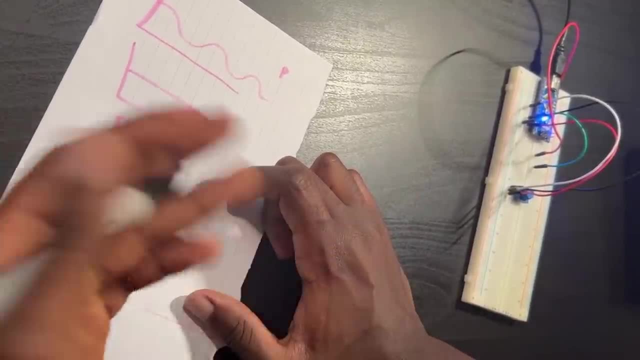 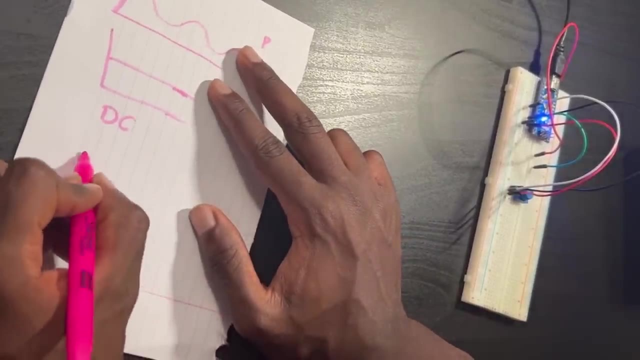 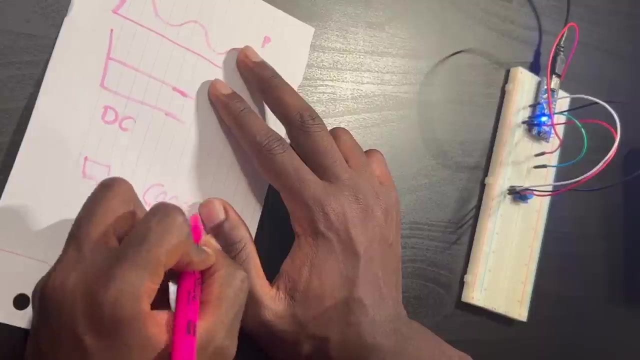 let me just explain this in a simple term, not get into too much detail. so what basically happens is this: okay, let me just bring a sharpie right here. basically happens this. so you see this, let's just see: there's a magnet right here, okay, and there's something it's attracted to right here, okay, there's. 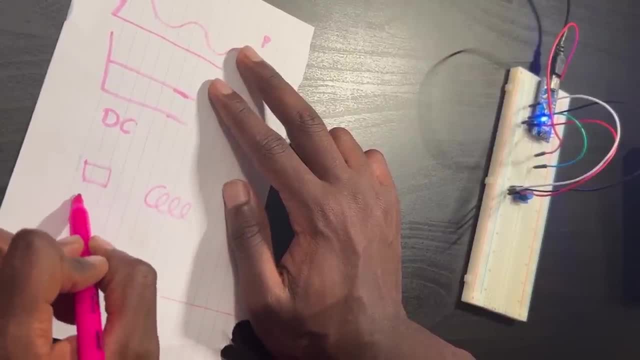 a magnet here and there's something it's attracted to. so when it's on, what happens is what it goes: attracted to, it's attracted to it, it goes right here. when it's off, what happens is what this magnet is repelled. okay, this magnet repels okay. so you see that it goes on and off. so basically what? 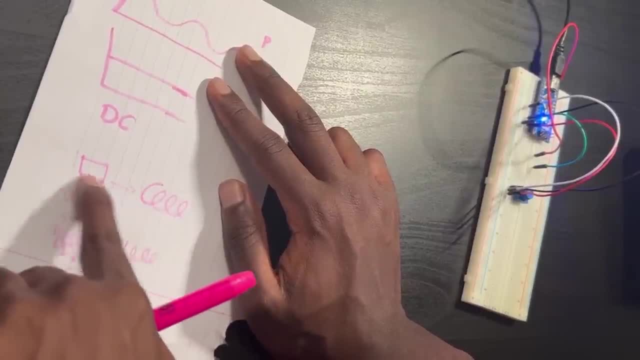 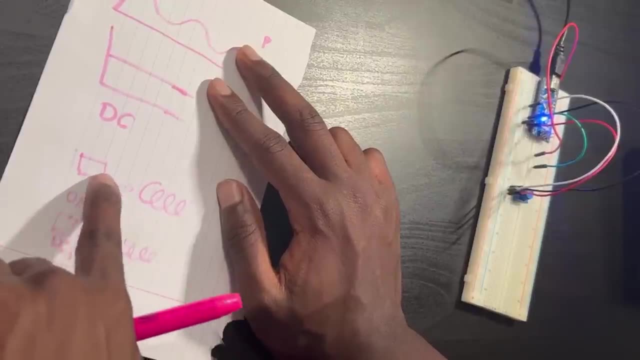 when it goes on and off at very fast speeds. what happens when it goes on and off and on and off? what happens, even using a dc circuit, what happens? what happens is it moves what back and forth. the vibration cone moves what back and forth, back and forth, back and forth. okay, so that's the whole essential thing. 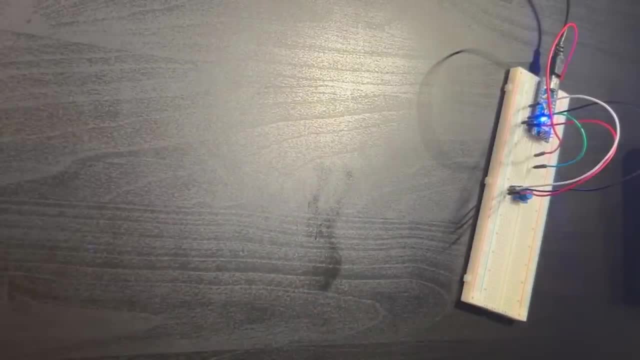 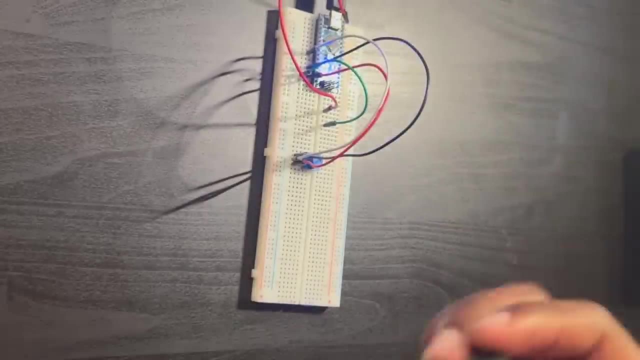 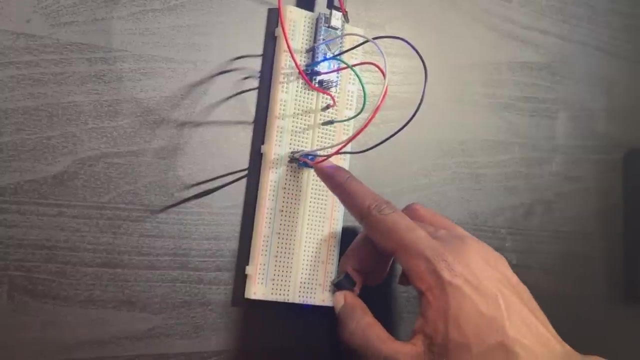 there's a vibration cone and it's moving what back and forth to create what vibe reach okay in mind. actually, let me just go right here. i have my uh, uh active buzzer right now. let me just go over to my active buzzer. what i'm gonna do is quite simple. i just want to create something that adjusts the. 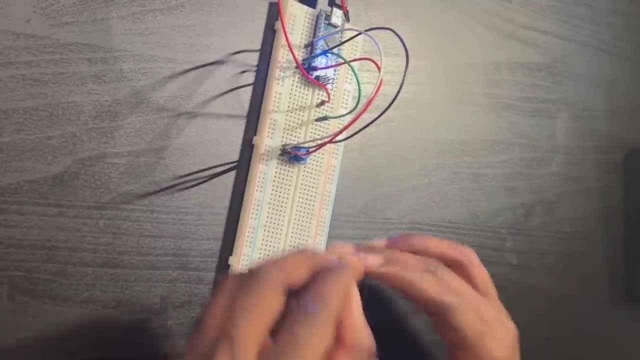 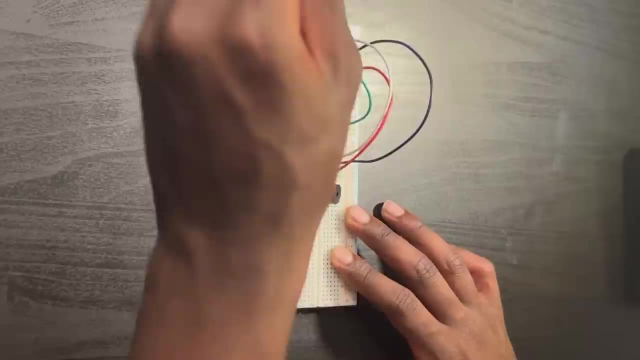 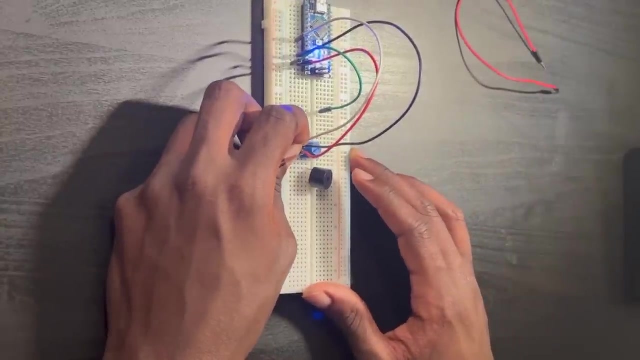 volume. so let's just use a potential meter right here. so let me just go back to my uh buzzer- again the positive size right here. so what i'm gonna do is let me just bring my connecting wire and what i'm going to do is i'm going to use this middle pin right now, the v, out of the potential meter. 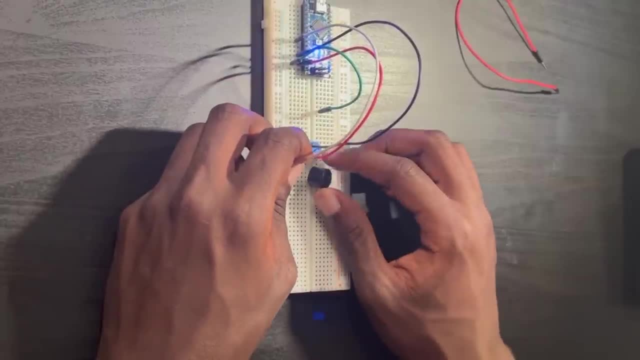 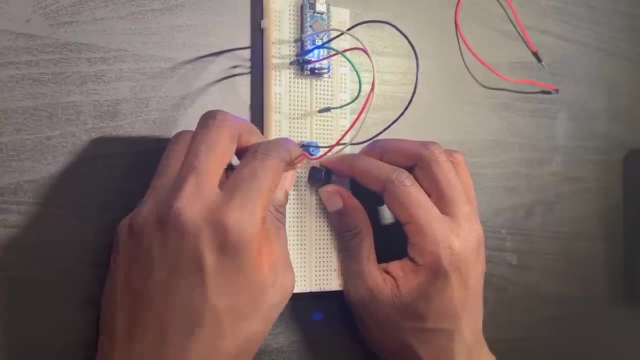 that we mentioned earlier. i'm just going to use this as my main terminal, okay, because then i can do what i can: adjust the voltage that comes out. okay, i'm just gonna adjust the voltage that comes out. okay, i'm just gonna adjust the. Okay, I'm just going to do that, and I need the GND pin. 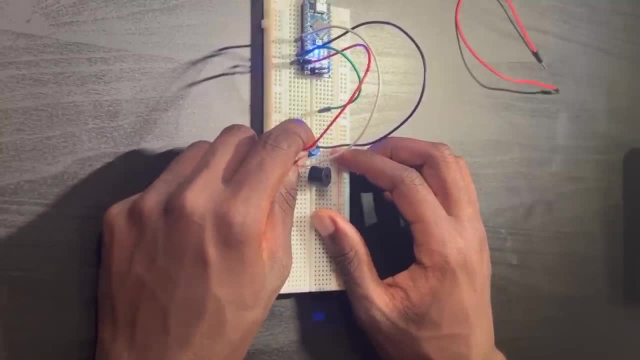 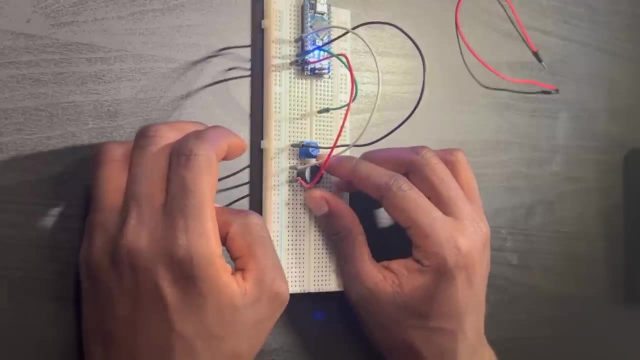 So obviously, I'm just going to take this GND pin from here and I'm going to put it at the end of the circuit. Let me just do that Now. it's supposed to work, All right. One thing I did not do is what. 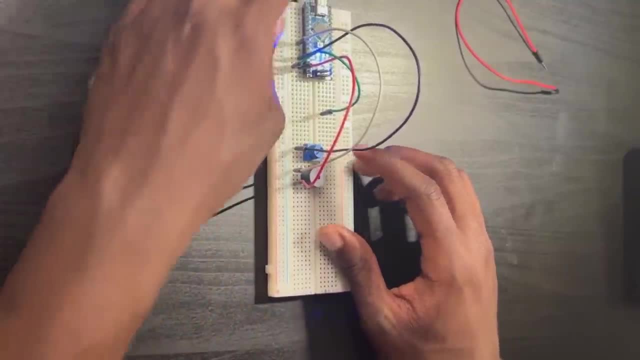 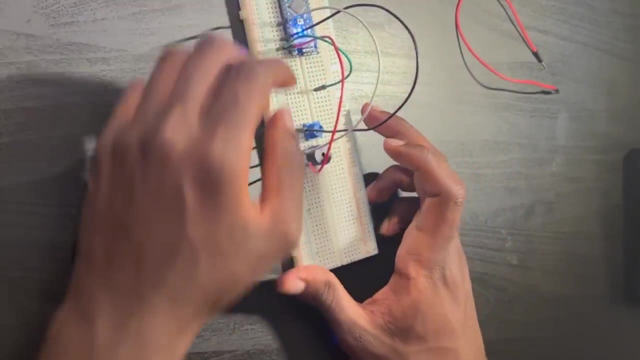 Right, what did I not do? The black one is supposed to be connected to what? To 5-volt. Is it connected to 5-volt? All right, so one thing I did is what I forgot about the potentiometer. 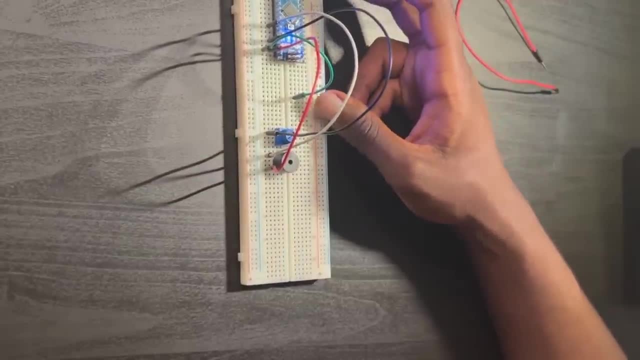 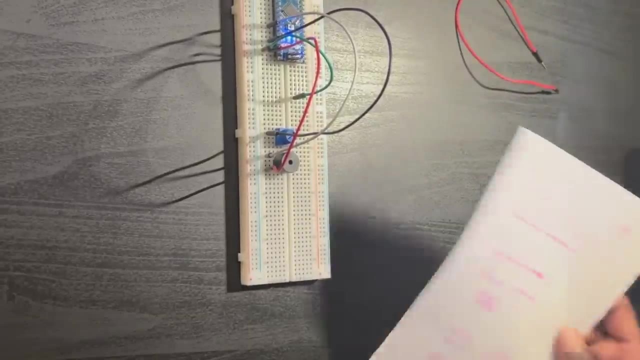 It's now what It has- to come from one end to the other end. Let me just again, if necessary, let me just draw the potentiometer again- Flip the page right now And, as I told you guys, let me just try to draw the circuit here. 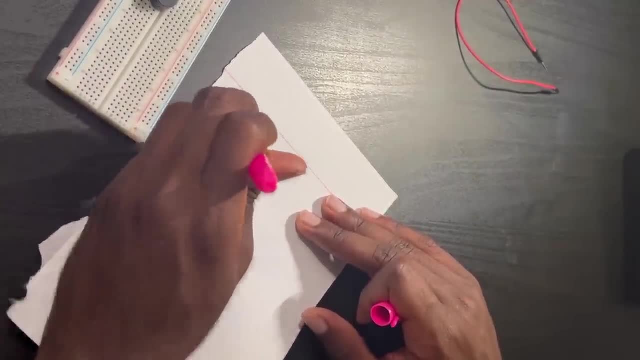 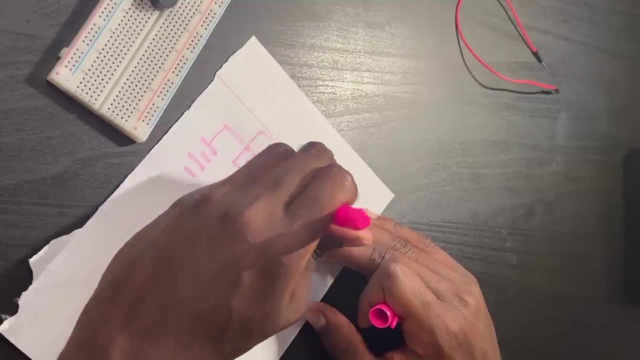 Okay, we have the battery- 5-volt. We have the potentiometer. It's what A box that has what? Two, Two resistors Connected to what In series. And in the middle we have what? 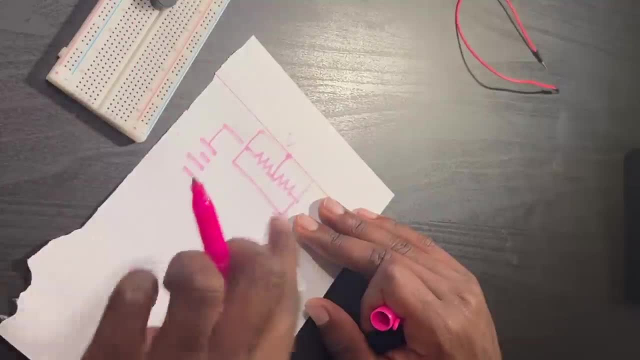 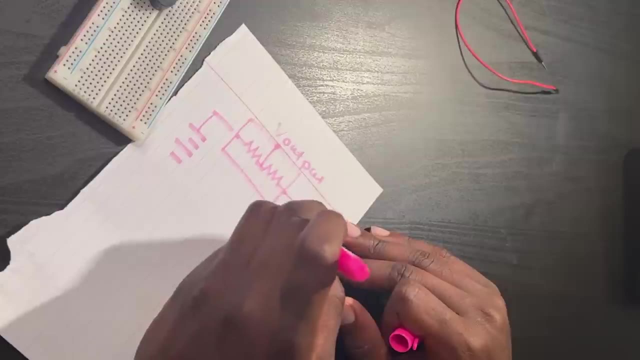 Something that's going to output our voltage. This one is like the what, The white pin, in this case The output. And we have what Afterwards? we have our buzzer that needs a positive side- Okay, a buzzer, And then it has a negative side. 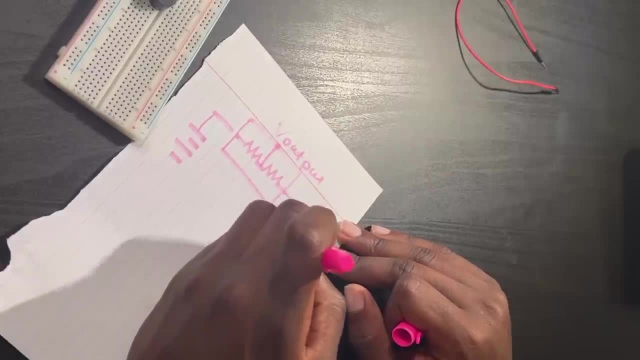 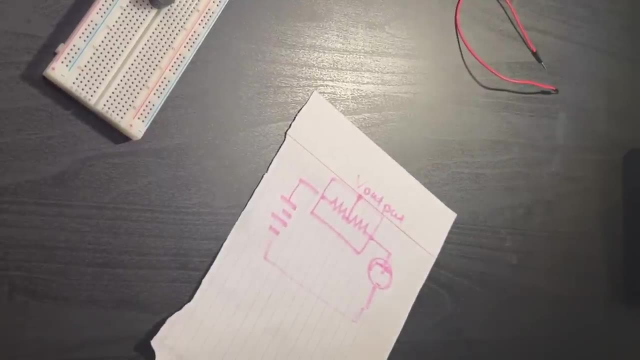 You just put it with a circle on top. It has a negative side. And then what We connect it to? what The negative side? Basically the what, The GNE. So one thing that I not do here is what. 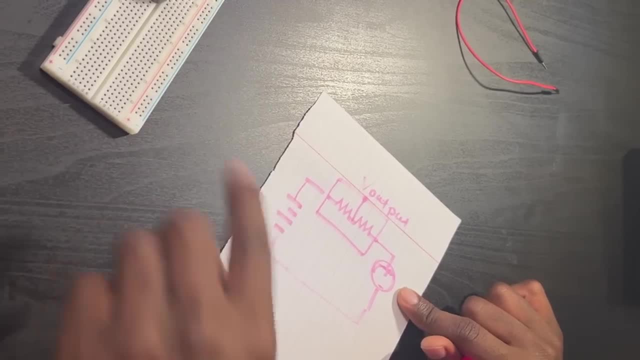 Connect the R2.. The R2 is right here. I did not connect it, I just jumped it. So what I need to do is like this. So let me go back right here, The V output. let it stay right here. 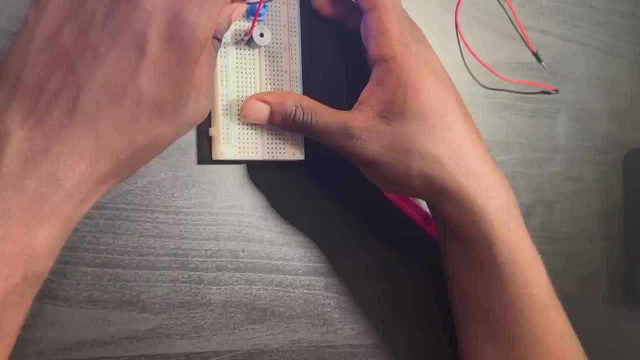 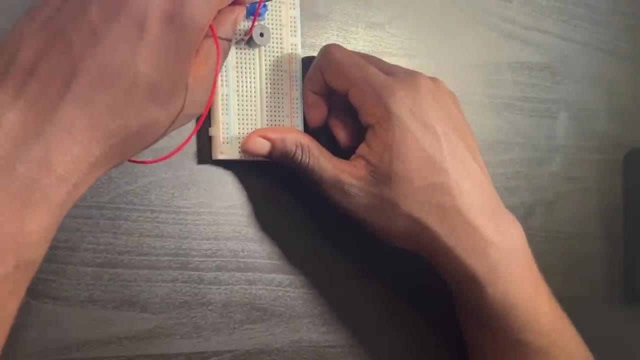 That makes sense, doesn't it? So you know what? I'm just going to put the V output right here. Okay, Then what? I'm going to need another wire to extend it. Just do that, Okay, Okay, Alrighty. 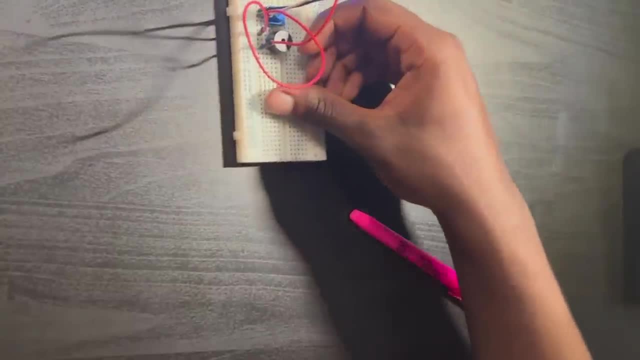 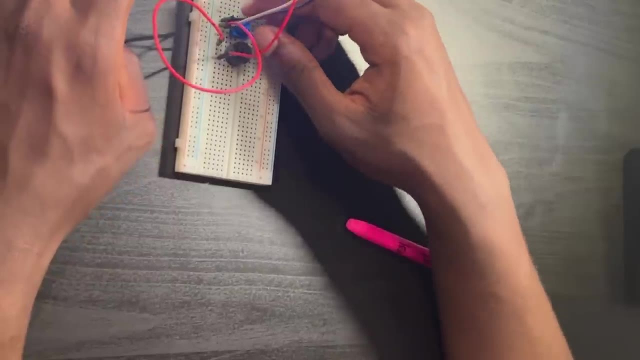 About to extend it. There you go, We extended. So we extended it on the what On the white pin: Basically, what, The middle? Okay, All right, So let me just try to adjust it a bit. I don't know if you can hear me, but let me just try to adjust it a bit. 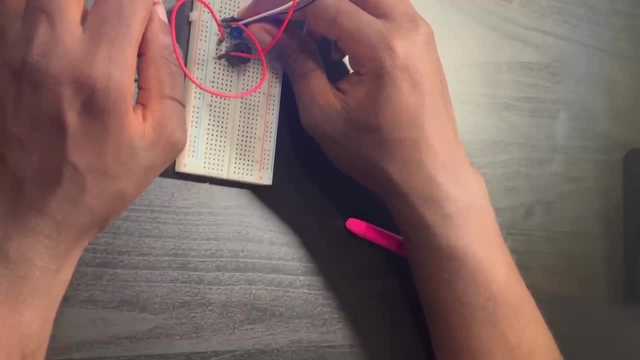 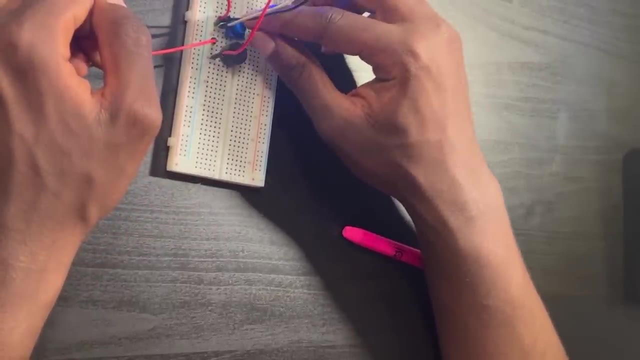 Okay, Let me just try to adjust it. Okay, I connected what- The white pin. I extended it to what? To the red pin. If you can see right here the white pin is the one. The V out is extended to what. 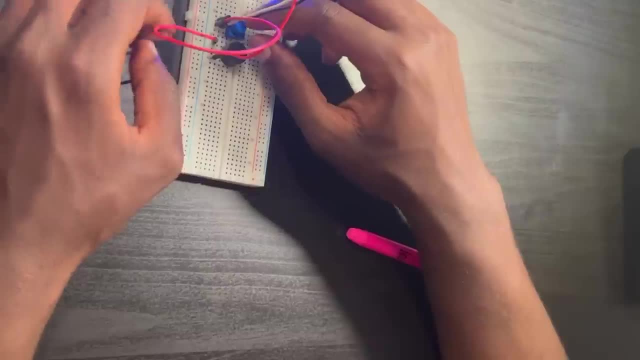 To the positive side of the what, The positive side of the buzzer. I'm using a what An active buzzer. again, Let me just try to, you know, use it as a turning knob, Basically use it as a volume adjuster. 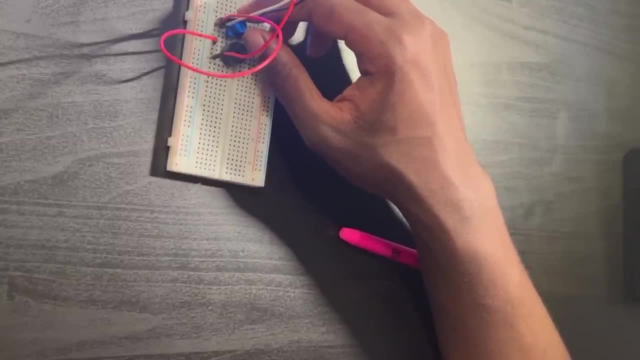 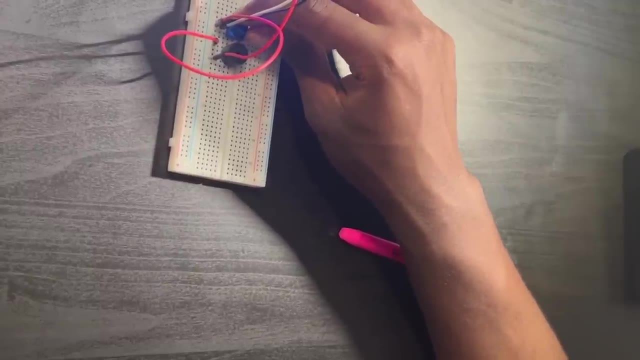 So what happens is you can barely hear anything at the middle or at the start, And then you can hear something at the what, At the very, very, very end. Okay, When I put it to the very end, Okay, Basically, when it's what: 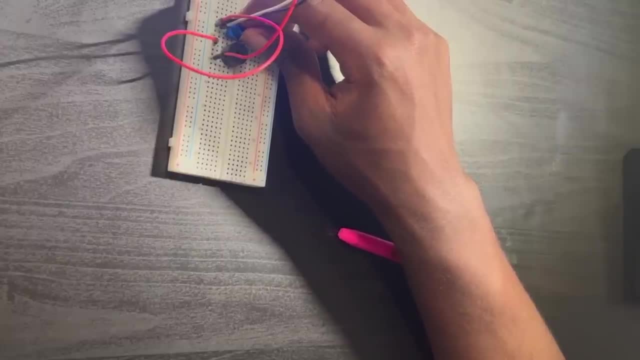 When it's receiving the maximum voltage, Basically almost 5 volt. It's receiving the maximum voltage. You see It doesn't make any sound when I turn it all the way. So obviously for this case do we need what? 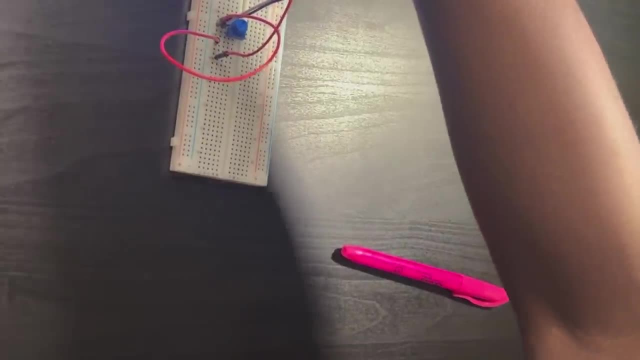 We need a passive buzzer. So let's just try doing that with a passive buzzer. So, instead of using what? Instead of using the 5 volt pin- again, I need to take it out of the 5 volt pin. 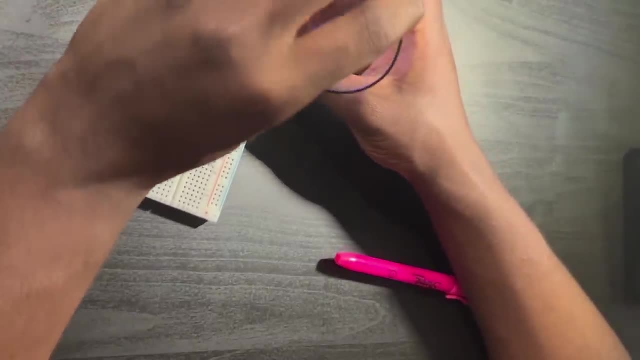 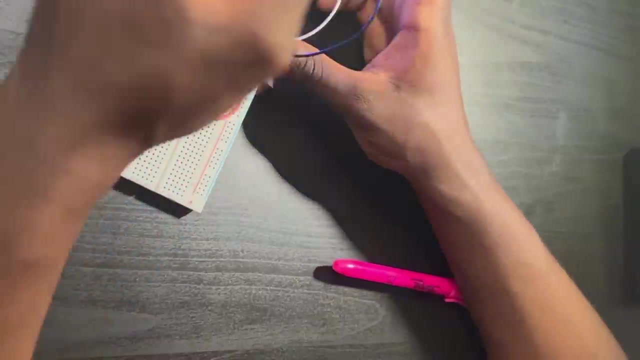 The 5 volt pin is connected to what? This one, This one, And I'm going to be using digital pin 9 instead. Okay, I'm just going to be using digital pin 9.. There we go, Then I'm just going to have my passive buzzer here. 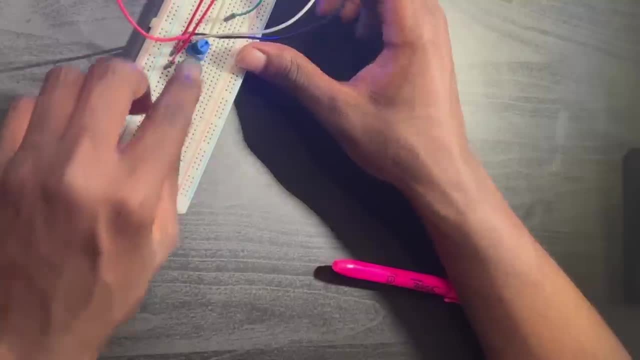 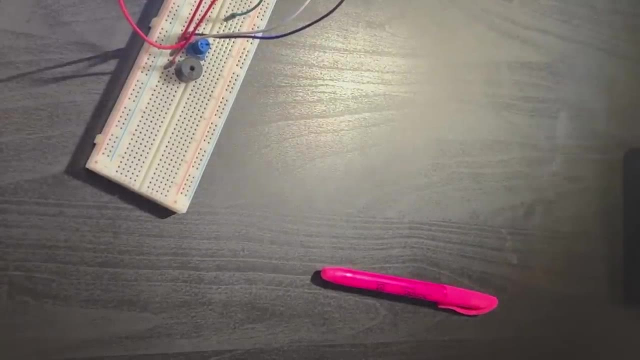 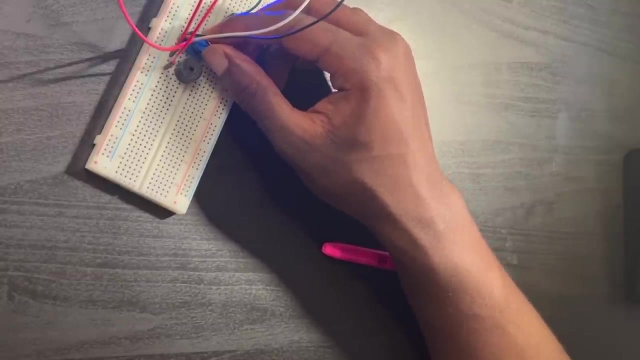 The positive and the negative side again marked. Okay, Now we should have what We should have: a voice adjustment. So let me again. what I'm going to do is right now, I'm just going to change it. Hopefully you can hear it now. 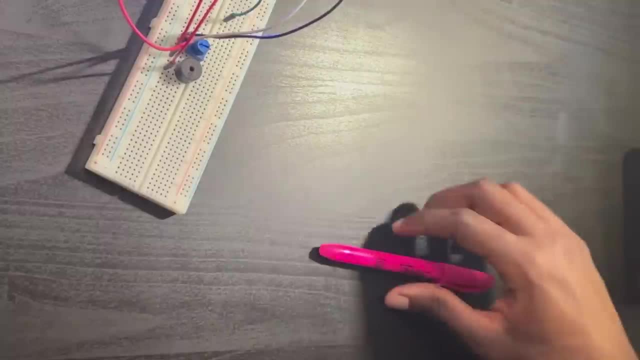 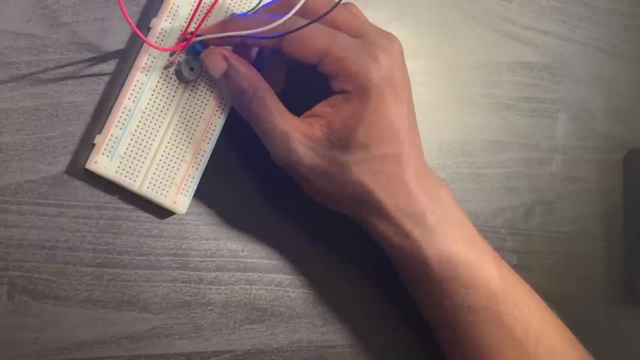 I'm just going to go silent And let's see the volume change. Can you hear? It's not the smoothest change, but definitely you can notice what the change in volume when it just changes. All right, Let me just go. 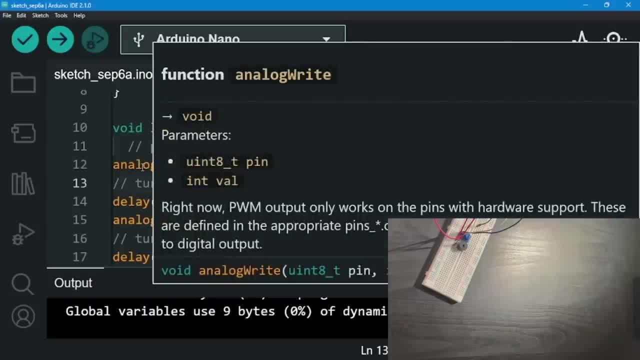 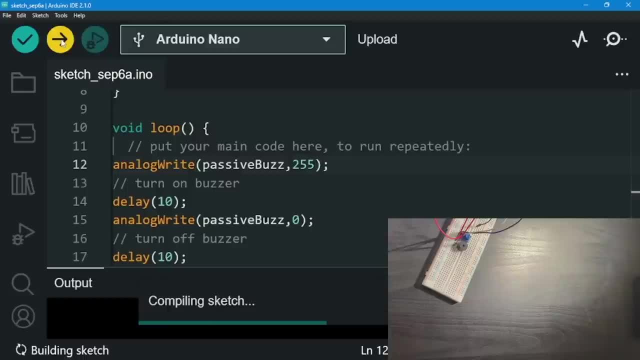 Let me just go right here and just give it more voltage. right now, I'm giving it maximum of 50.. Let me just give it 255, which is the maximum value. Let me just give it a maximum value right now. Okay. 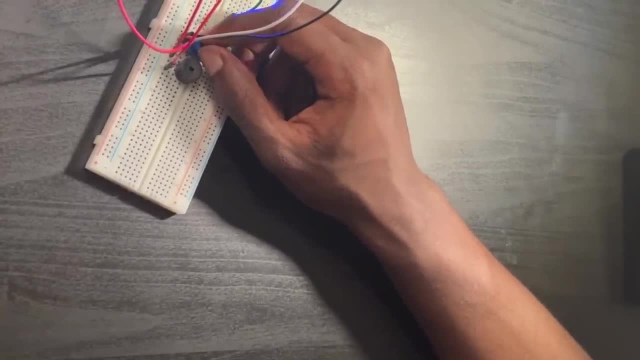 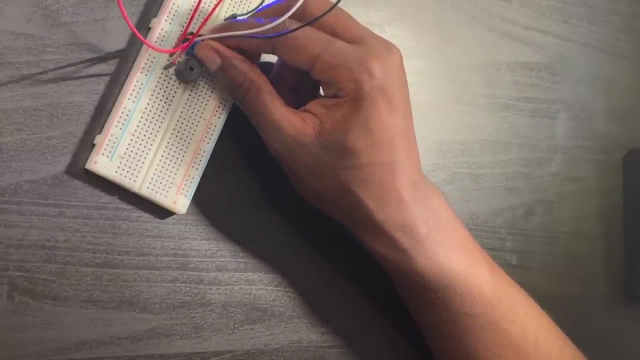 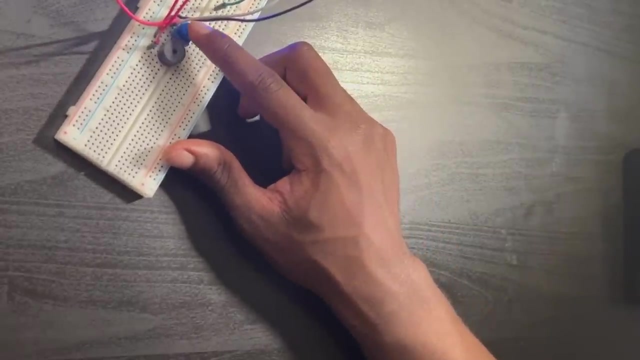 So now let's just adjust it again from here. Can you hear? Now it's what It's basically. the potentiometer is what. we're using it as an adjuster, All right. So again, potentiometer, we use it as what? 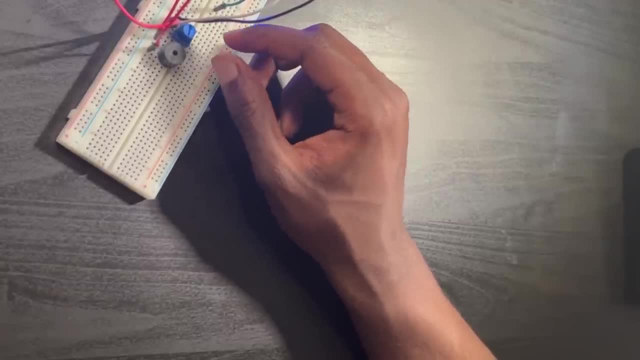 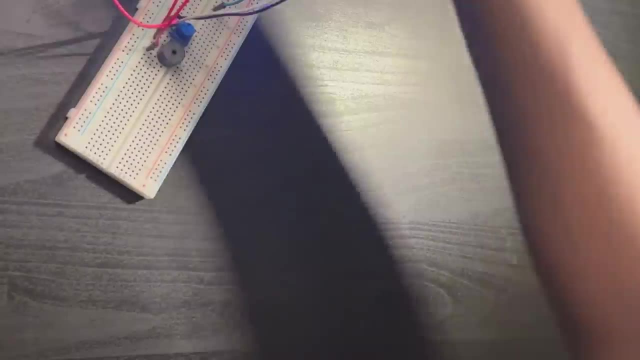 As an adjustment, basically as an adjuster for what? For the amount of voltage that comes out, Basically the current, the voltage that comes out. Okay, So we used our buzzers right now We used the passive buzzer. i have the active buzzer here. we're not using it. we're using the passive buzzer, right. 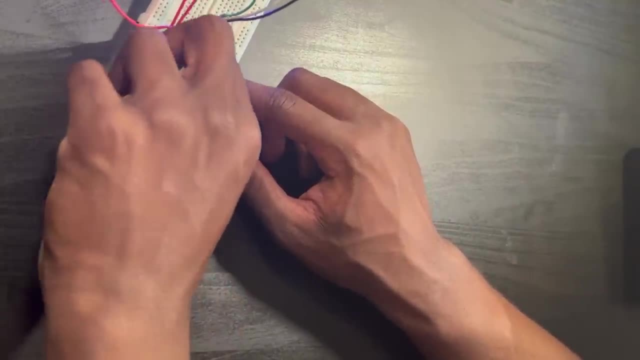 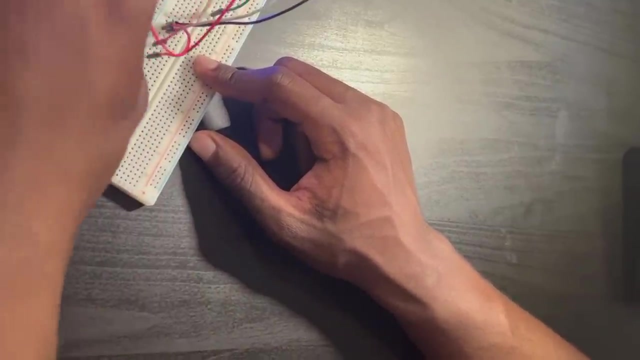 now. so we made this simple project okay. so now we learned about what we learned about these buzzers and how to make really really good songs with really good sounds, with all right. so even then too, if you actually let me go to my screen right now, let's make this a bit more interesting than 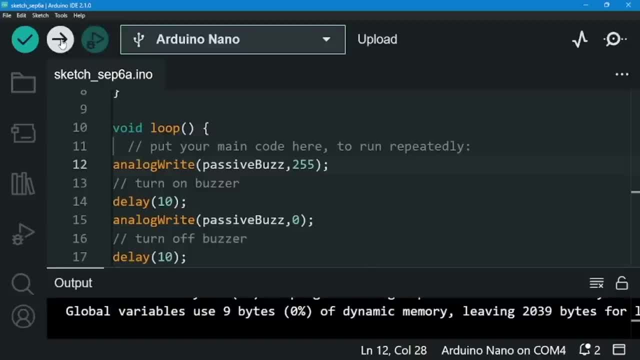 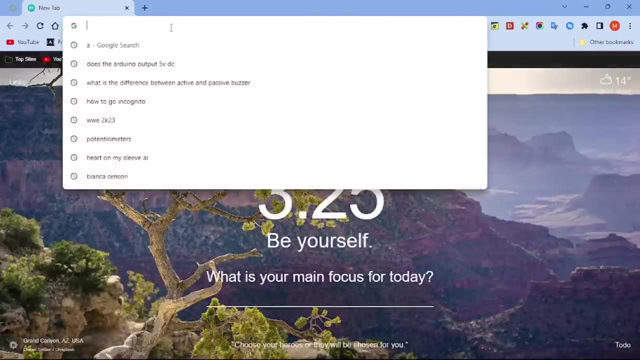 it is. so let me go over to my screen right now. okay, i don't need all these wires right now, let me just remove them. i don't need my potentiometer right now, let me just remove them, okay. so let me just go to my chrome right now and if you go right here, let me just say buzzer, buzzer, arduino. 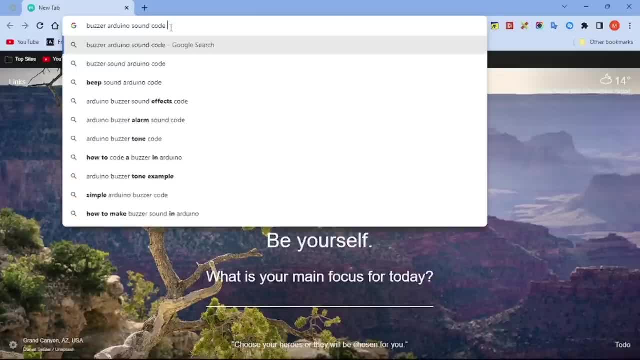 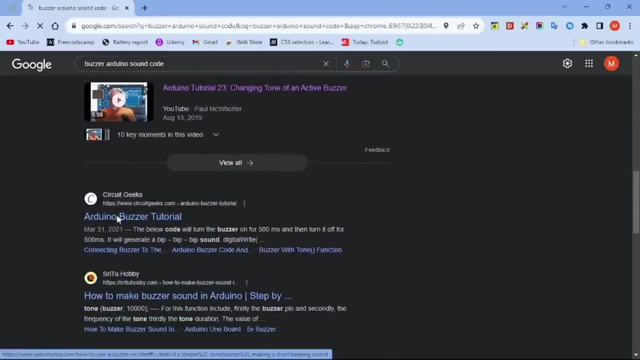 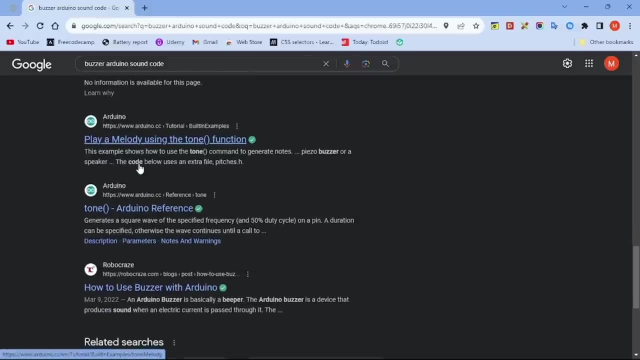 sound code. it'll just go for a code, okay. all right, let's try to find a good code sound, all right. so there are going to be lots and lots of uh play a melody using the tone function right here. let me just again, let me just try to open this. but what you can do, what i'm going to, 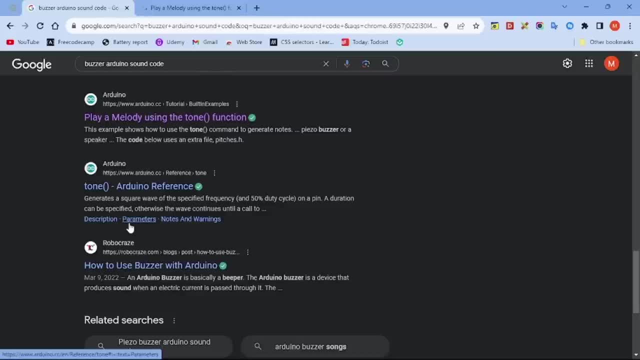 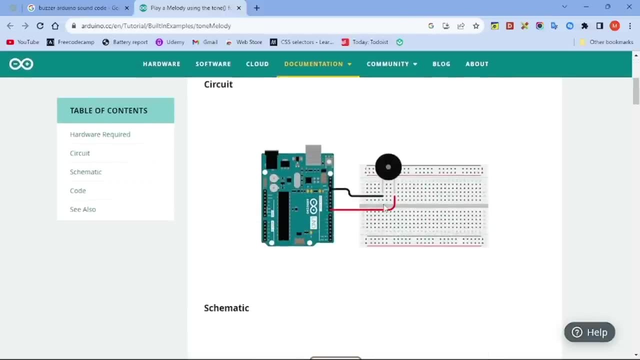 give you as a homework is what. what i'm going to give you as a homework is: try to find- all right, try to find- these arduino codes again that use a buzzer. you can see that right there we're using a buzzer right now. right now, i don't know what buzzer we're using. i don't know if you're connected to a. 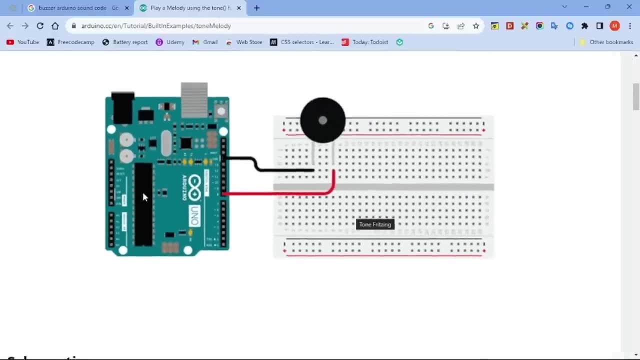 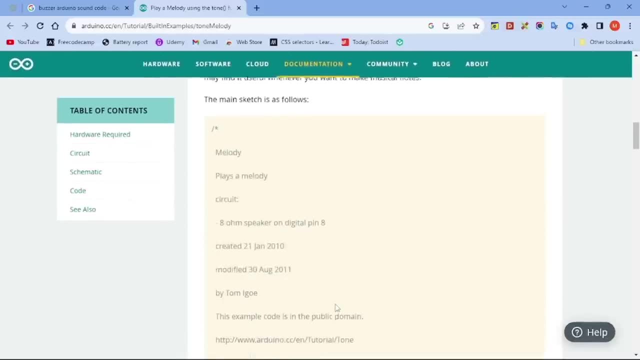 pin or a 5 volt. the image is not the best. all right, let me just go here. okay, there we go, we're connected to the pin and then we're going to go to the arduino code and we're going to go to the pin 8 and gnd. okay, all right, and there's the. there's the code right here. all i need to do is 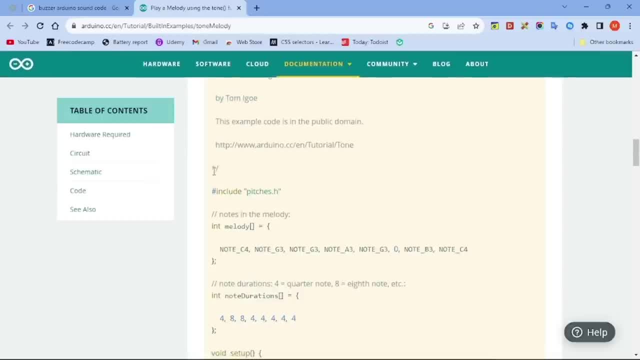 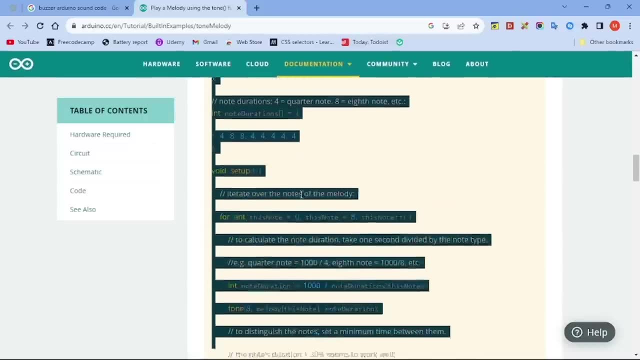 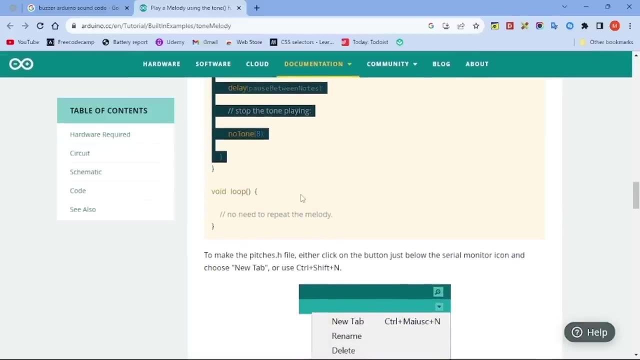 what? let me just copy the code right here and it has a library. i need to include that, and i'm actually going to see how to even include libraries right now. so let me just copy all of this. okay, i'm copying all of it. all right, there we go. no need to repeat melody or whatever, just 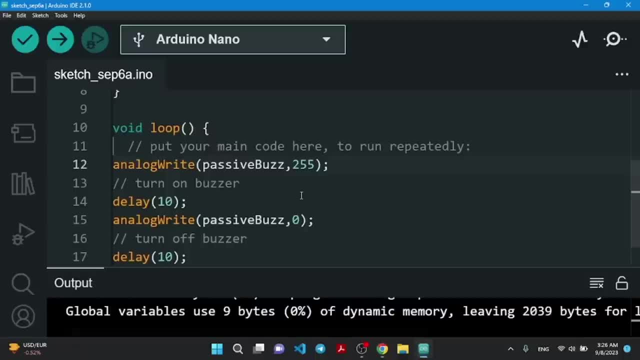 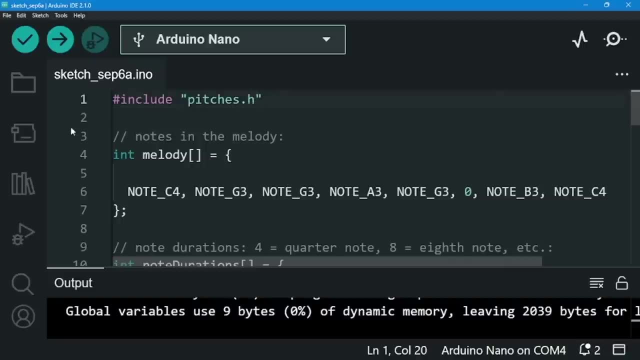 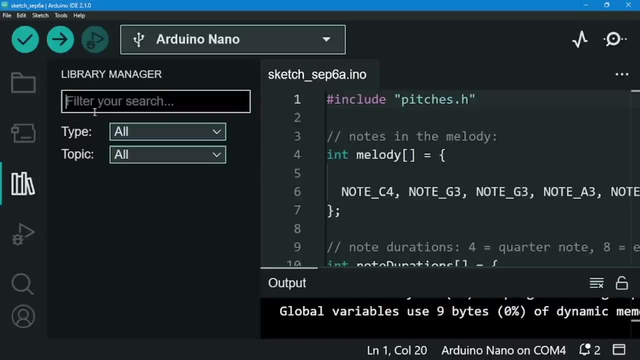 copy this right now. let me just put this: yeah, paste this fully, and one thing i need to do is what? install a library. okay, there's a word manager. you go right here and there's a library manager, so let me filter my search. i'm just going to say pitches. 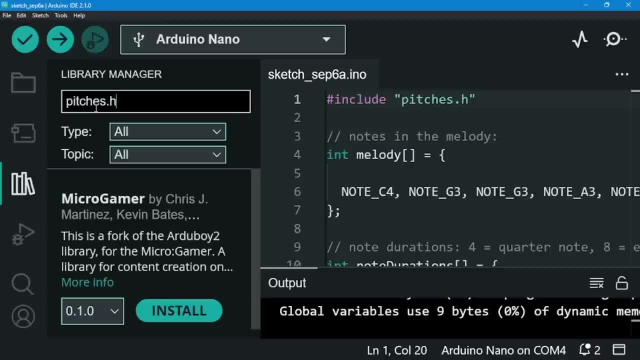 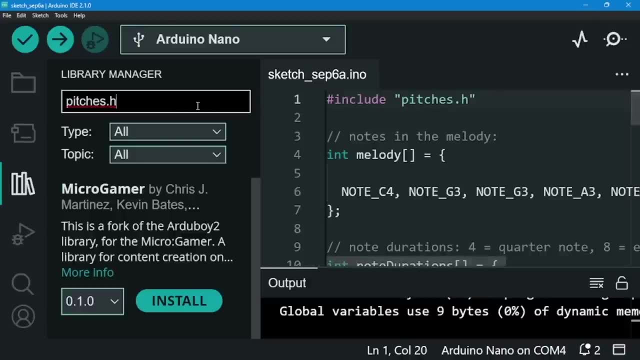 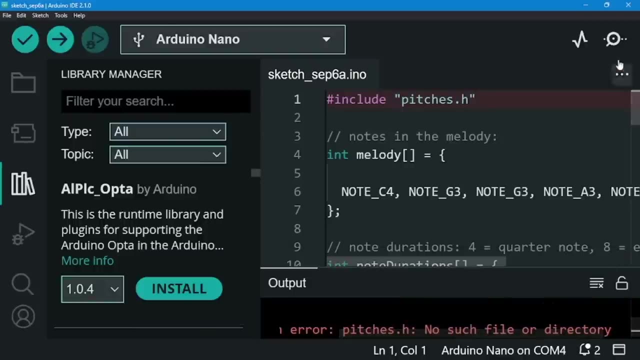 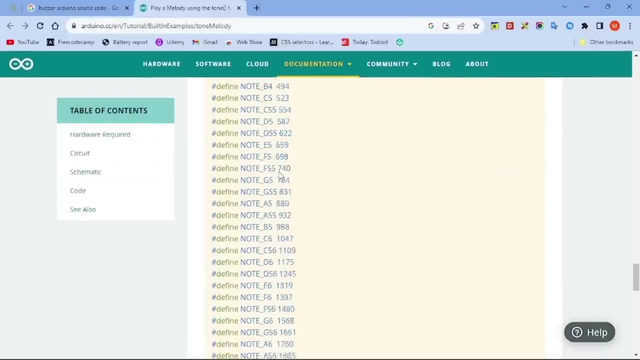 okay, this is micro gamer. just go and try to even run the code before. uh, including the right. let's see what? there's nothing called pitches dot edge, okay, so let me just try to google it right here. one of the pitches dot edges. there are definitely lots of notes, as you can see right here. let me just go to the. it just stopped. 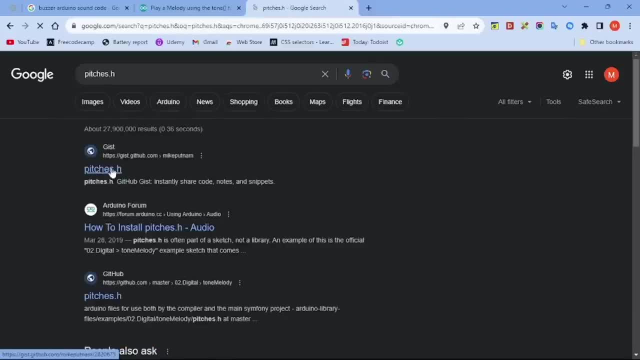 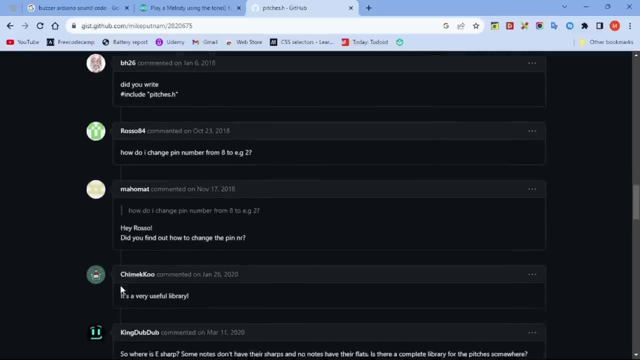 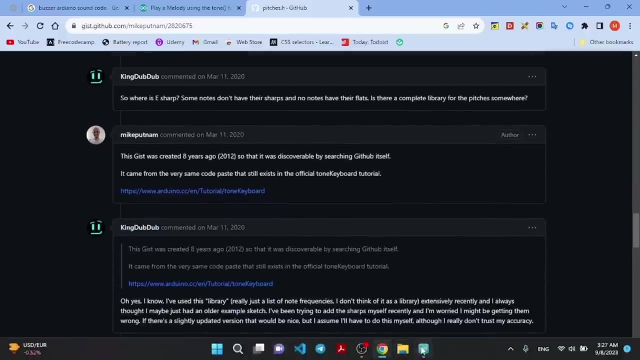 there we go. yeah, we're getting to its github page right now. it's just dot edge and i'm trying to include it as our uh, there we go. so i'm trying to include it in our library right now. i'm trying to encode it in our library. as you can see, right now i'm trying to search for. 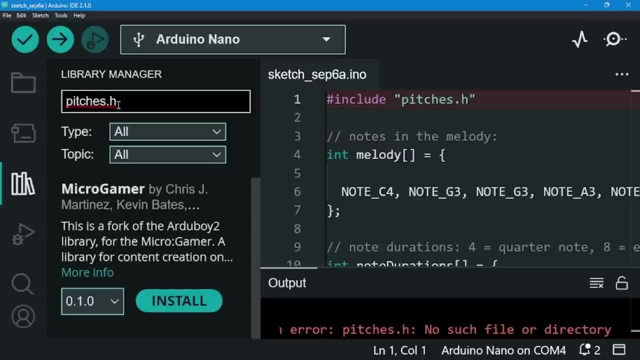 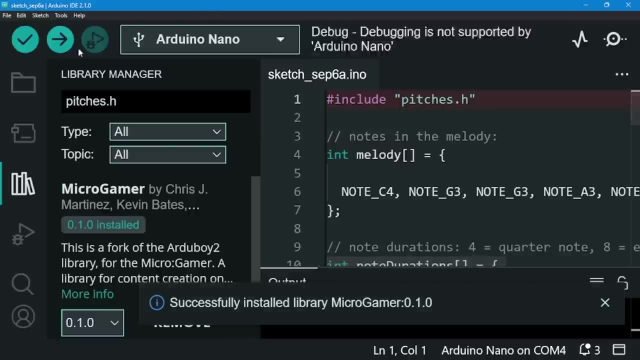 pictures: dot edge. okay, it's just not edge, just do that. so again, do it yourself. again try to go to problems and do it yourself. okay, let me just install this, because don't miss coming in here. okay, let me just install this and let's try to verify our code. even that too, if it actually 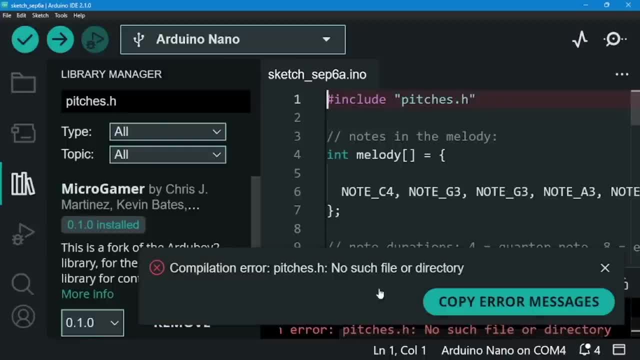 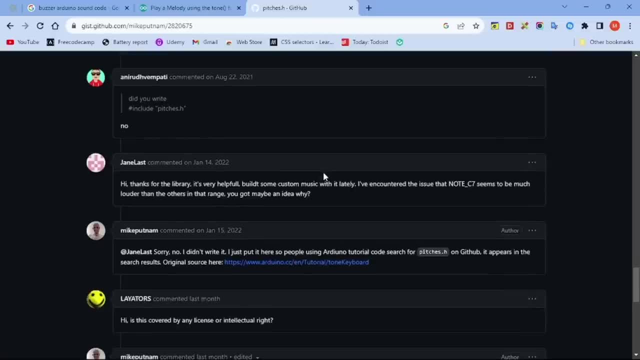 works all right. it says: there's nothing as in this directory. no file in this directory. okay, pictures, dot. edge. there's nothing in this directory. that's what it's basically saying. so what you need to do in this case is basically simple: okay, so what i do in this case is just: 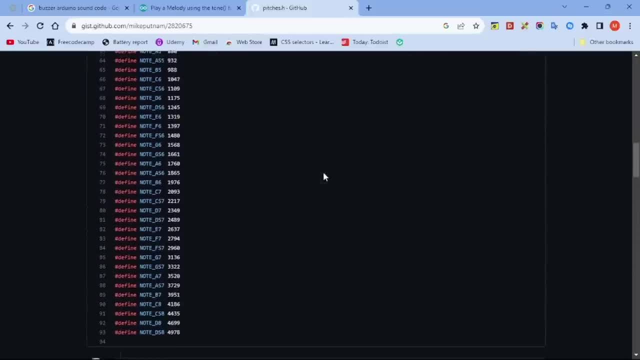 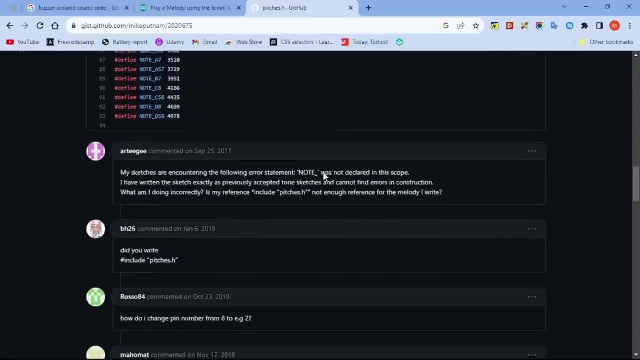 go to github or any other documentation and ask them a simple question. okay, i don't know how to you know, include libraries at github or any other documentation? so i'm just going to go to my directory and C++, because I mainly use it. So, all right, let's just go here. 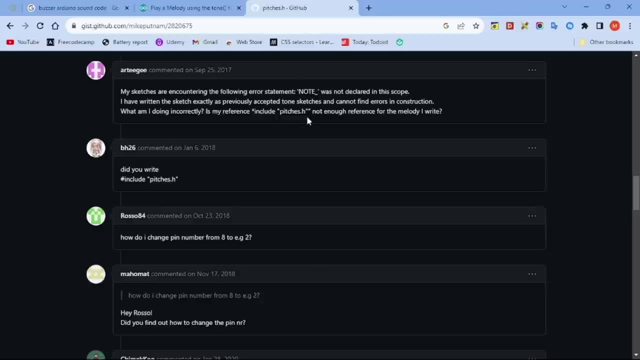 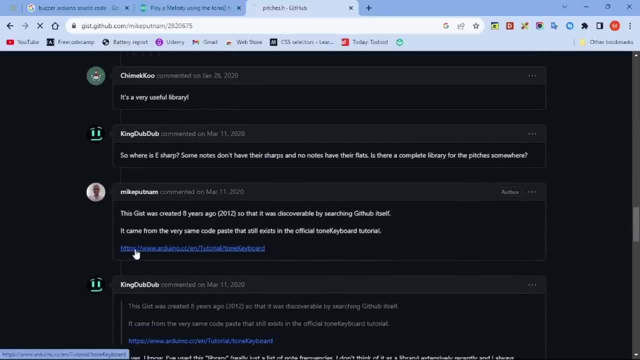 My sketch is uncovering the following error: I just don't. it's not enough. Okay, reference, Try to read. one Leads me to this link Right now. this leads me to this link and it doesn't seem to go any further. 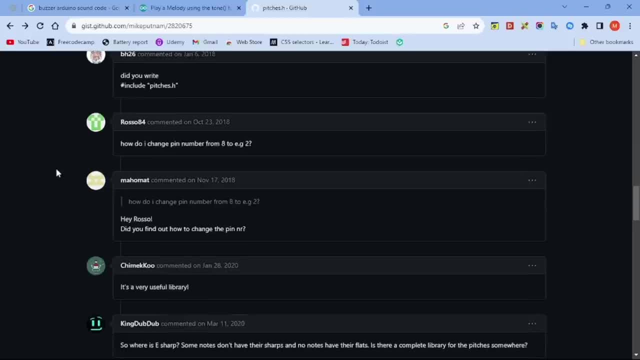 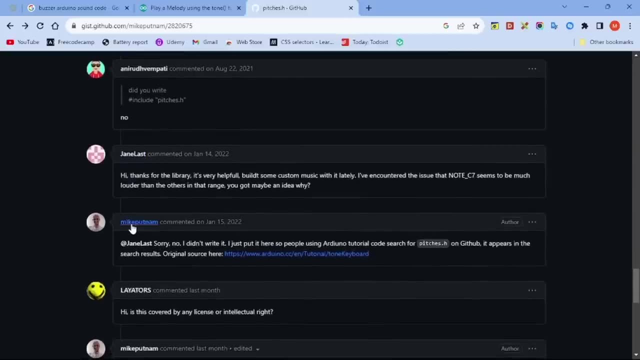 Okay, then how do we do it? How do we go and add library store on Arduino? Okay, because I used to know this, but over time I think I forgot about it. All right, pitchesh does not seem to be working. 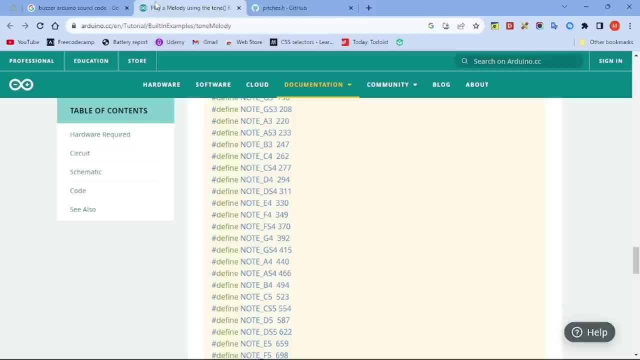 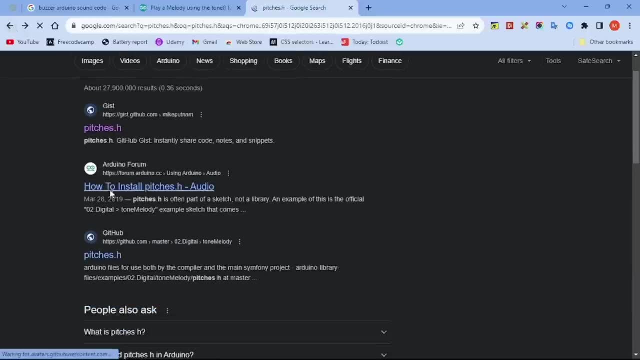 All right, so let's try to use something that does not have any library. But one thing: I'm going to go over this again: how to use libraries and stuff in the future. All right, how to install pitchesh audio, Let's just go here. 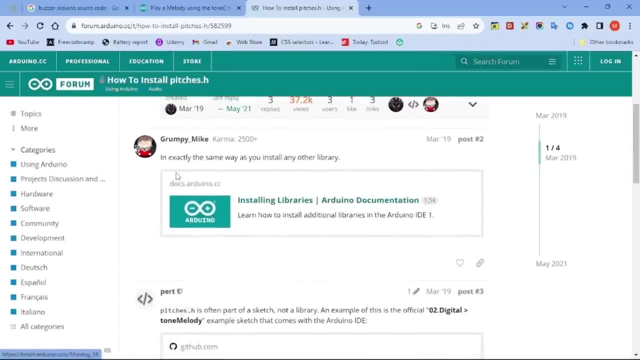 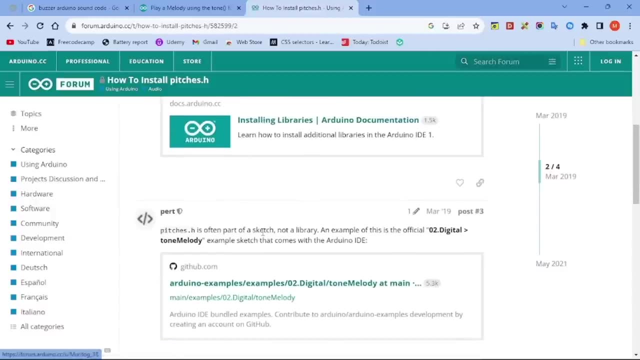 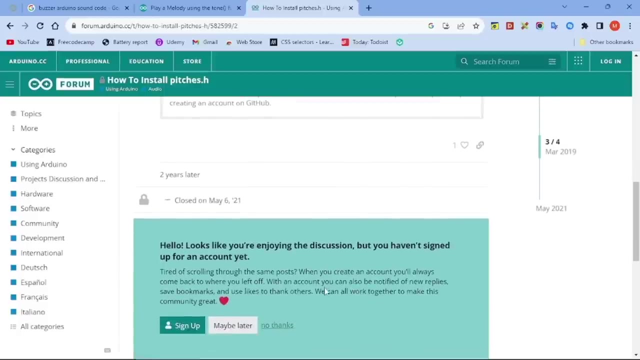 This is an Arduino form and how to install it. There's an Arduino documentation of what Installing libraries right here. Pitchh is a part of all right. zero two, All right, I haven't signed on. All right, so it's telling me to do what. 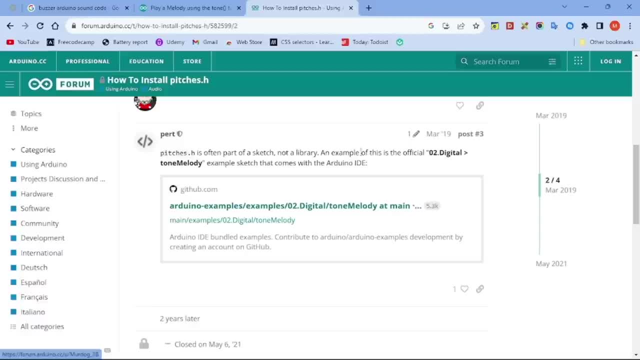 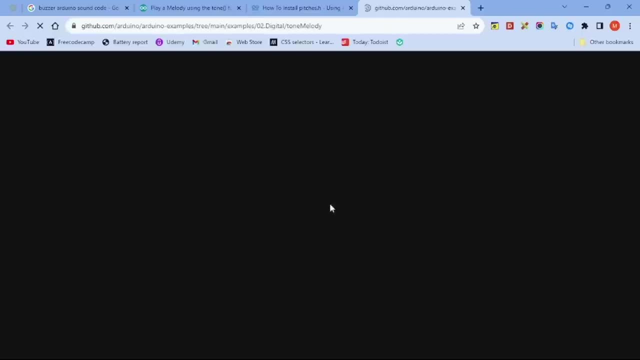 It's part of what- A sketch, not a library. An example of this is official 0.2 digital sketch that comes with the what With the Arduino IDE. All right, it's leading me towards this, So again, I'm just running to what. 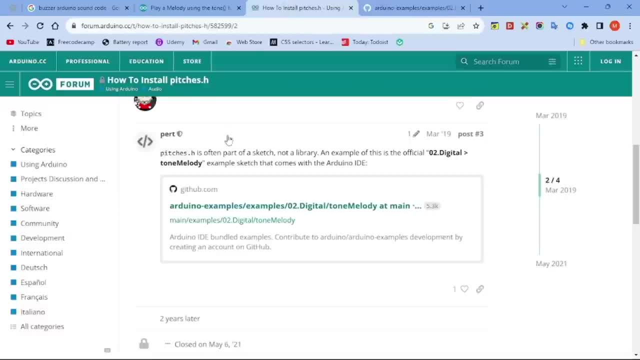 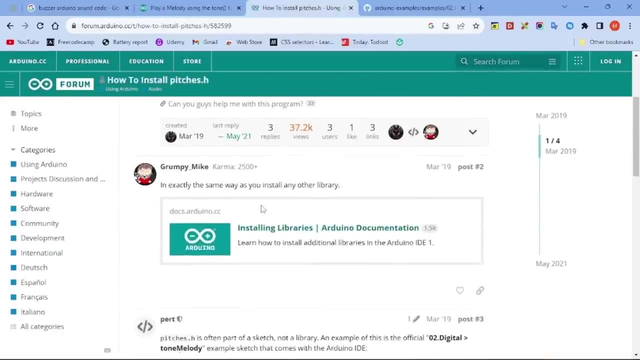 We're running towards the problem again. the same problem again. It seems that we can't solve it right now. We're going to need to solve it later on. Okay, let me just check the installing libraries documentation Again. I'm trying to do this together with you guys. 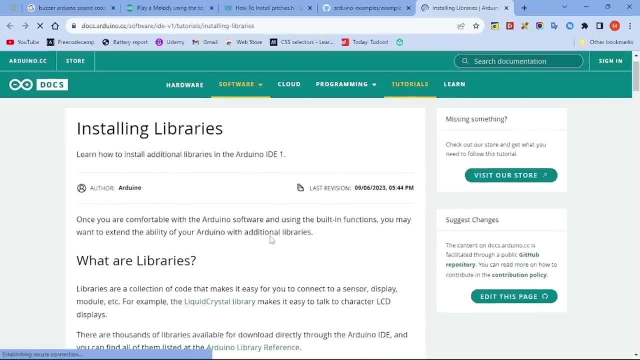 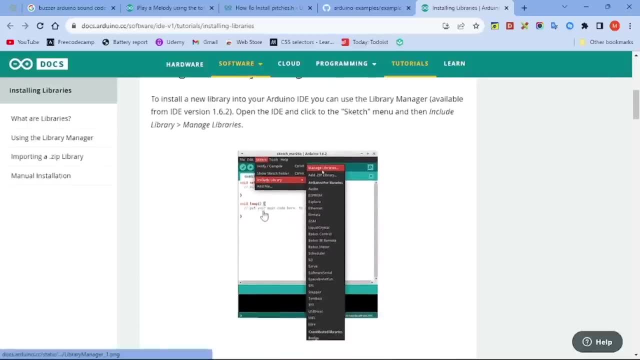 since what happens is with when it comes to courses, is it just seems easy when somebody else goes to the end? We don't. it doesn't seem that you're. you're going through a problem, We are, Everybody does Okay, All right, so let me just go to again. library manager. 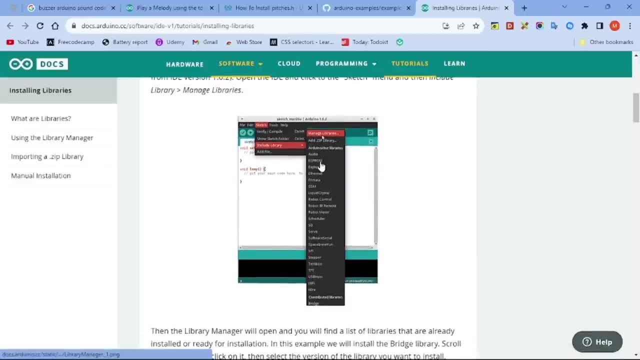 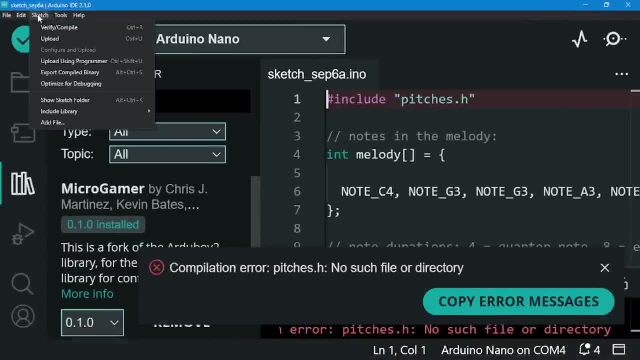 Let me just do that. So all right, let me just go to sketch: include library and manage libraries. All right, let me just do that Sketch. Let me see it's include library right now. I'm going to say manage libraries right now. 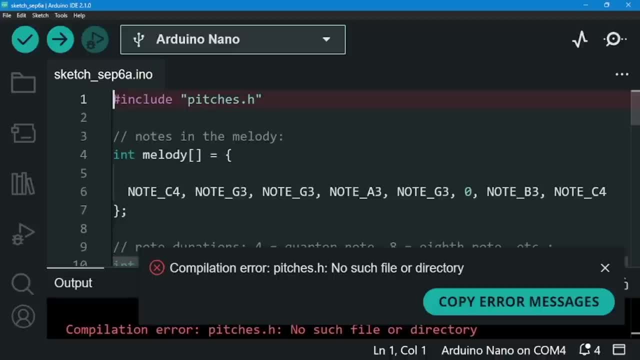 Okay, Open the tab right now. Okay, Let me just do that. Okay, Let me just do that. Okay, I'm just going to go again just to show you, to you guys Manage libraries. Okay, there we go. 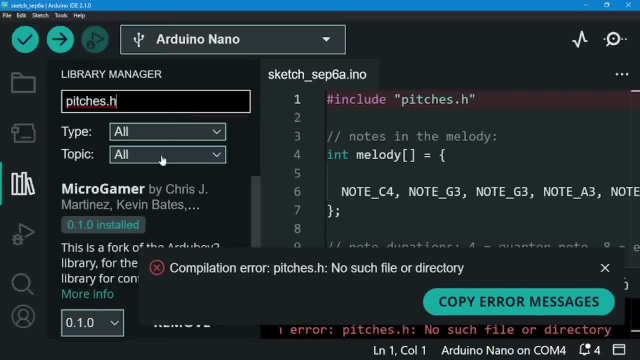 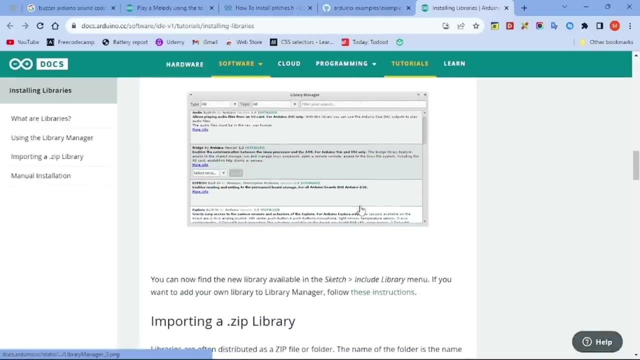 Just let me do the same thing. Pitches, The link of pitch, just shows me pictures. So it does not have a good document documentation, because if it did, it's going to show me, uh, basically how to even install it. you see that at adult zip library it can do that. so basically, what i need to do is what: 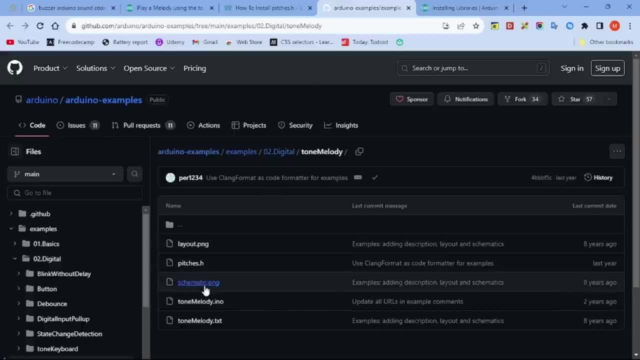 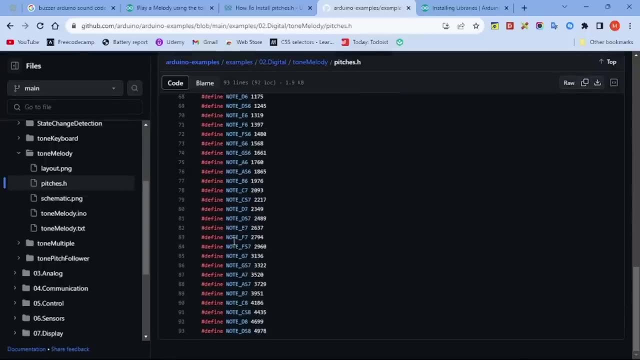 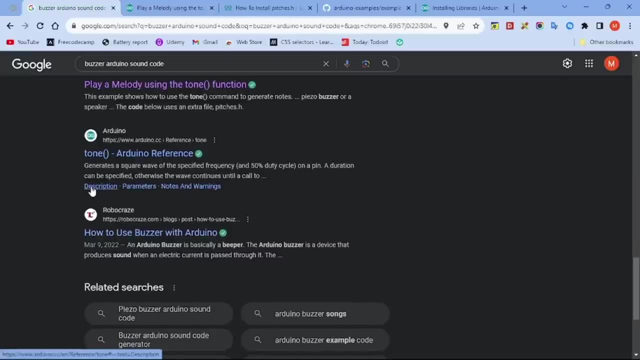 download this pitchesh right now. that's what it basically telling me to. i have to download this, basically this code, download this and run it. so let's just try to find something else that actually does not require me to do. what to use? this pitch is thinking: okay, so let's just say. 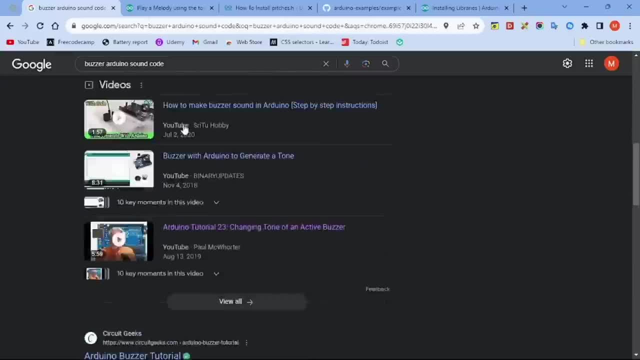 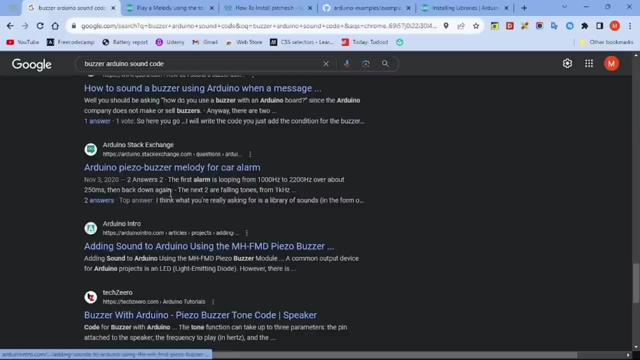 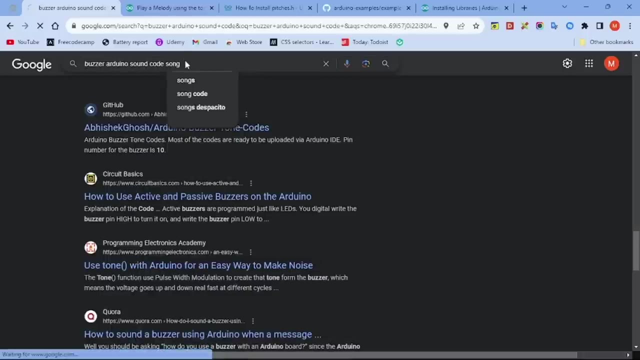 buzzer. arduino sound code. again, let's try to find it. this is part of programming, but you cannot find the things you actually want. okay, let me just say code. let's just say song song code. see that play parrots of the caribbean theme song on arduino. there are definitely lots and lots. 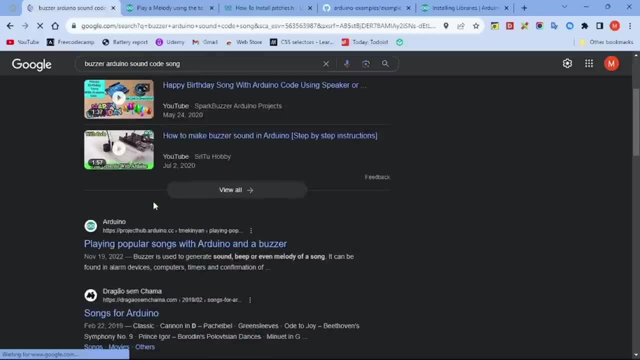 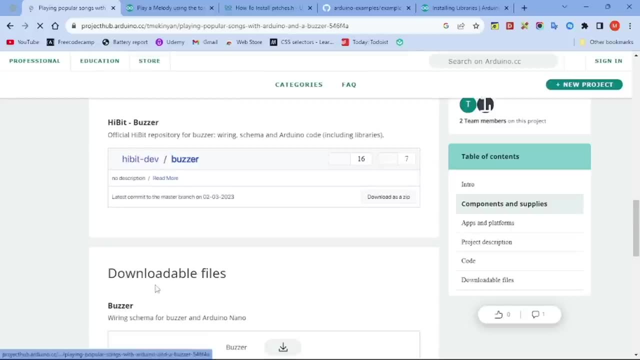 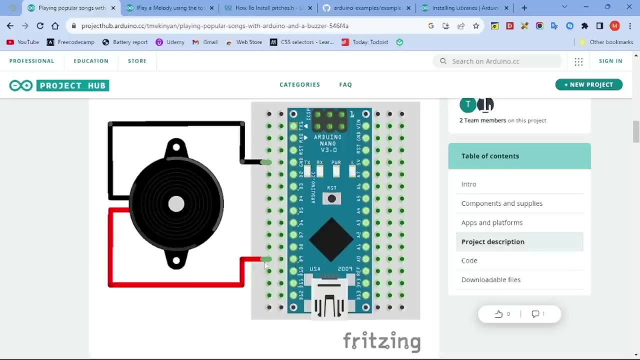 of great youtube videos again to actually make a. there we go, arduino and a buzzer songs for arduino. let's just try this one. all right, there we go. let's just see the component again. you have the gnd and be connected to pin nine, right? okay, that makes sense. you have to include the pitches. 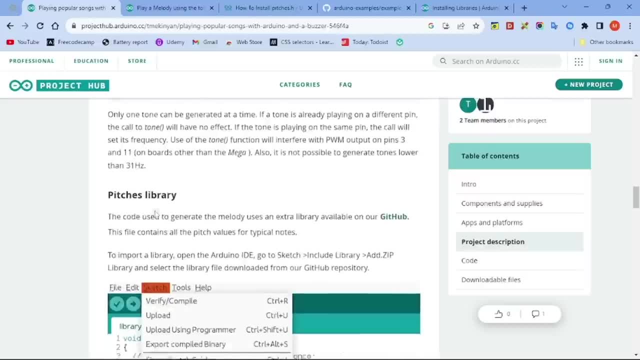 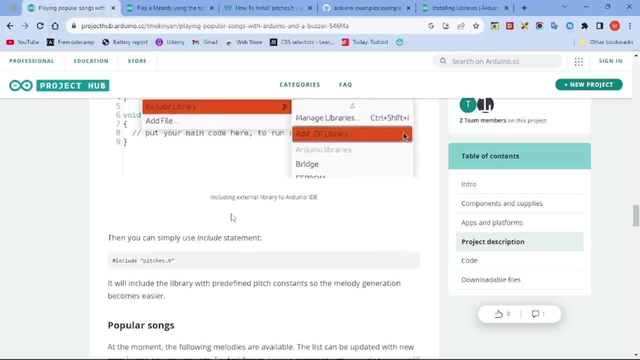 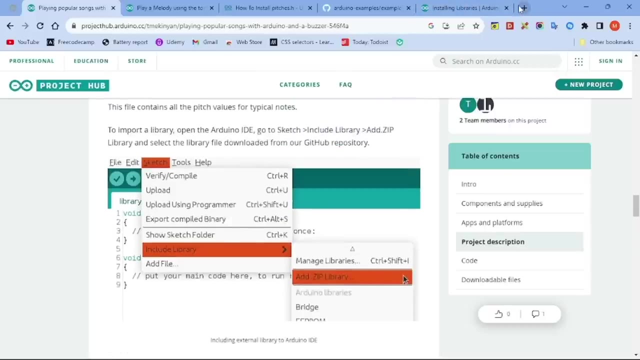 again nine. you have to do that. you keep using this library. okay, include library, add zip library, all right. all right, there we go add a zip library, but we do. we do what we definitely need: pitchesh what we need to download it. as far as i'm concerned, right now we need to what pitchesh i need to. 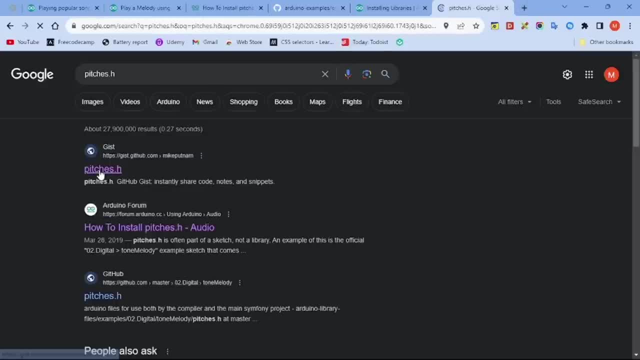 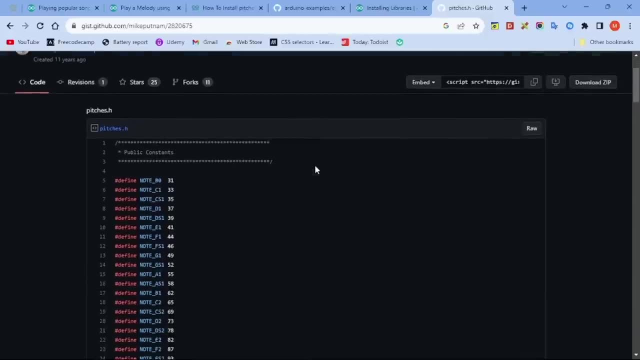 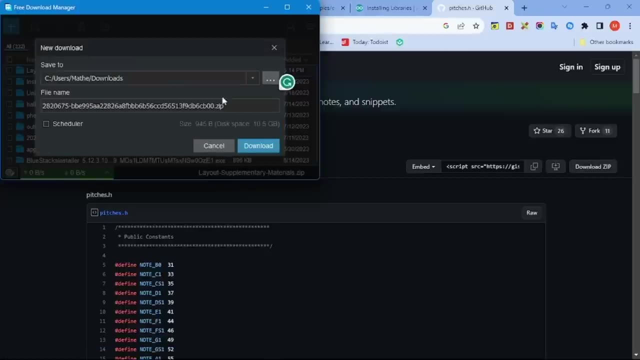 find the library and download the zip. let me just go to picturesh right now. i should finally get hung about it all. right, there we go, pitchesh. i'm just going to download this right now. let me just do that. i'm just going to call this pitchesh. 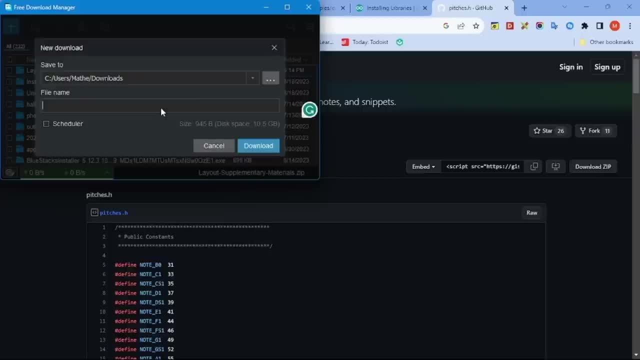 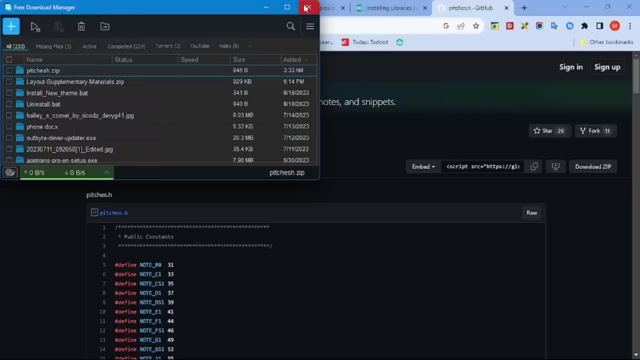 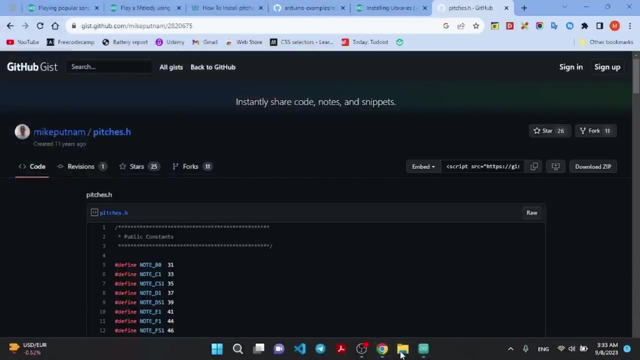 because it just makes more sense: pitchesh don't zip. let me just call it that. okay, that should be better, isn't it better right now? okay, so let me just do that, import that. let's try that. let me just import it. uh, how do i do that? 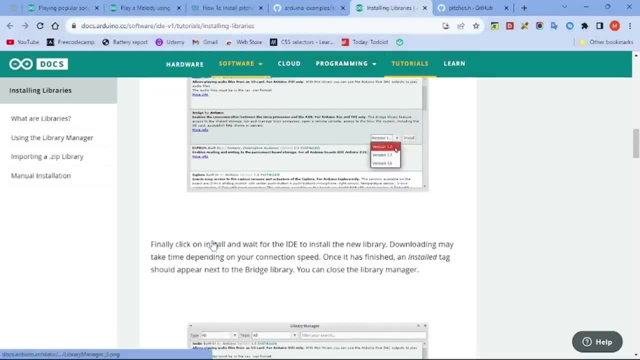 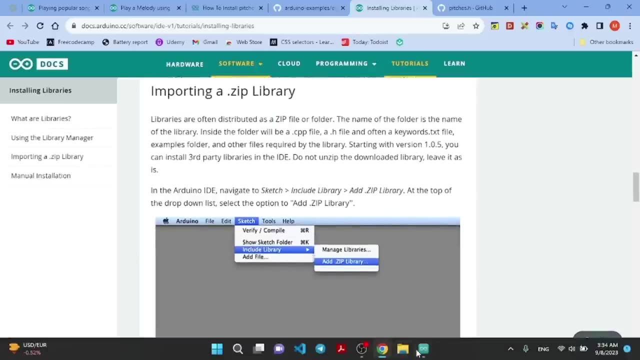 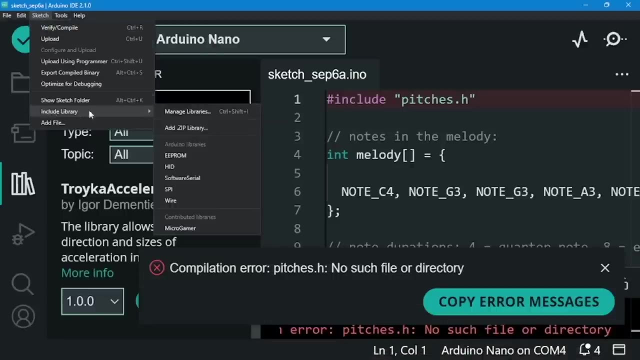 i go back to this tab, it's showing me how to import it. so, okay, i'm pointing this: zip library sketch in library, add zip libraries. let's just do that. so let me go right here. let's go tools, actually let's go to sketch and let's include library and then add zip libraries. it's not available in the. 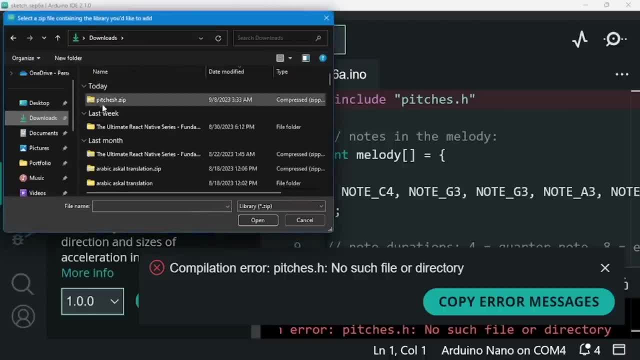 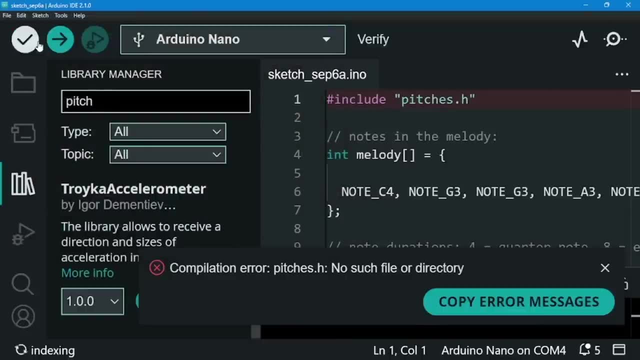 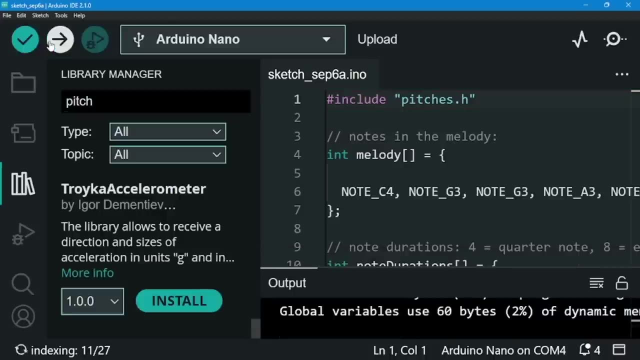 library manager. it's not available in the public library, but just edge. don't let me just try to do that. it's processing it and it's installed it, so i think my question is working now. hopefully it is okay. it's done compiling, so hopefully now it's gonna work. let me just upload it. okay, it's done compiling, so that's nice, okay. 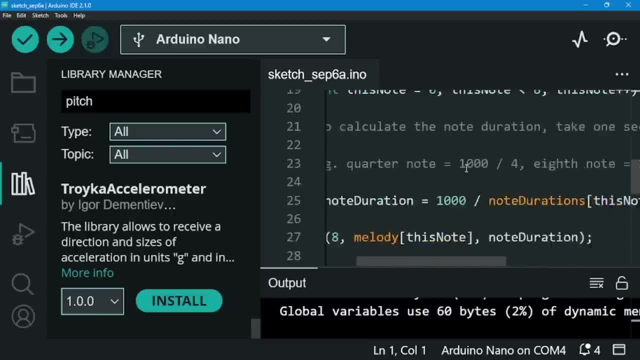 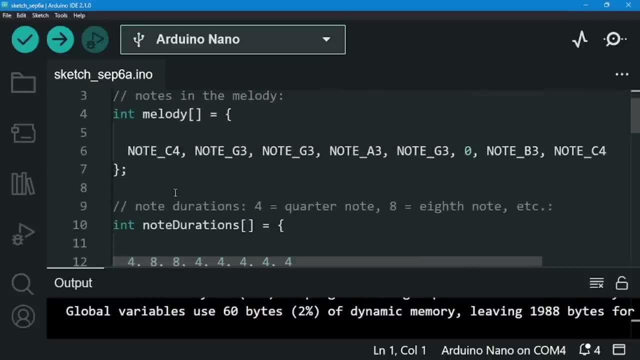 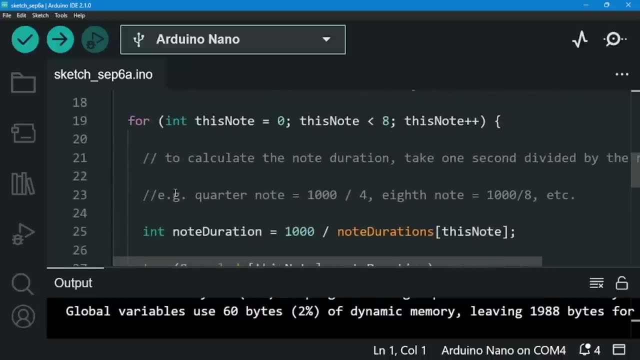 melody, can you see that? all right, so we used our library manager right here, but one thing we actually need is what it does not include what pin i use for this. you know, that's the problem right here. the problem i have right here is what it does not tell me what pin i'm supposed to use. 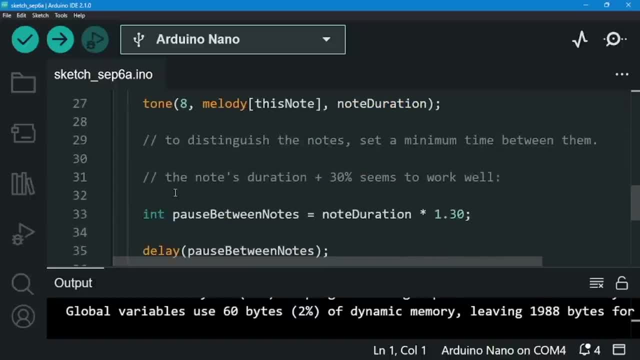 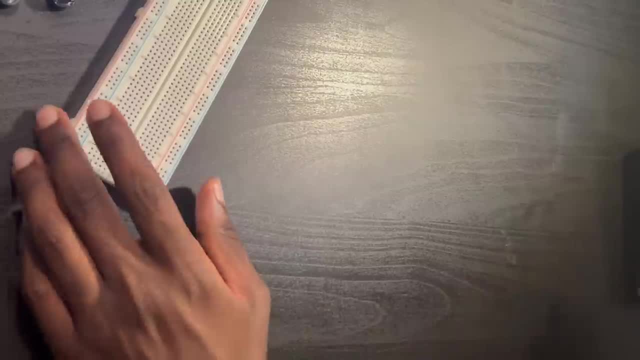 does it? does it even set up a pin mode? i don't think it does. i think in this case we're going to be using an active buzzer here because we're not setting up any pin mode, and all that for uh, for uh, for passive buzzer, so we're just 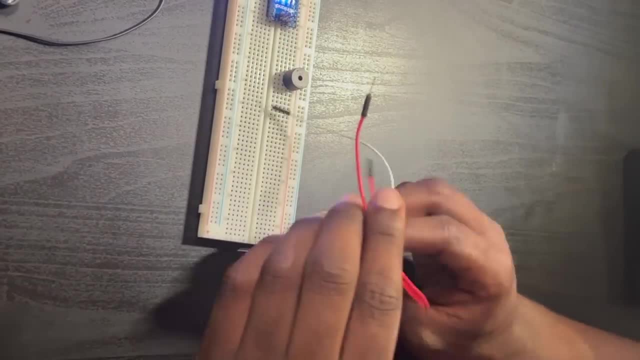 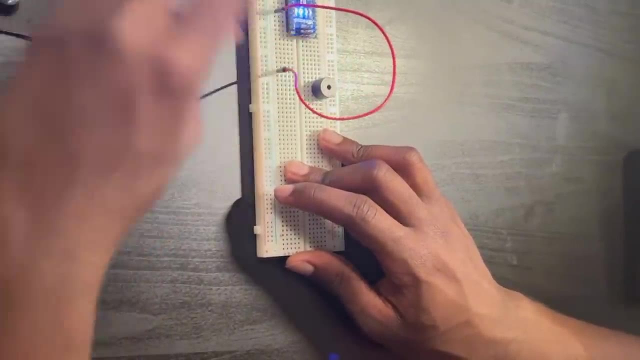 going to be using what i'm going to assume we're going to be using an active buzzer here. that makes more sense. so let me just connect the 5 volt right here. connect the 5 volt, let me just put it right here. and we have the gnd. let me just again connect the gnd right here. it's. it's a bit. 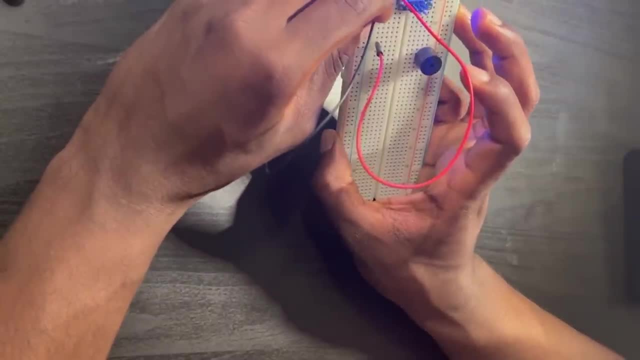 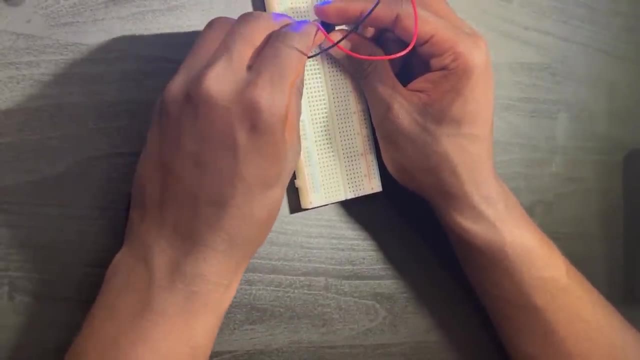 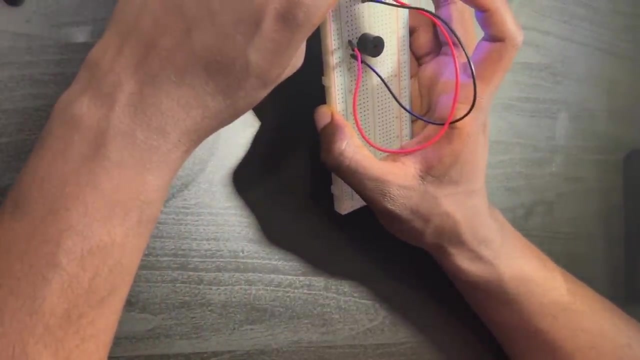 harder when you're filming it to actually get the right pin. let me just go over here. gnd got it okay. i think that's how it's supposed to work. let me just make sure again. i got the five volt and then i get the wrong pin. i think i did get the wrong pin. 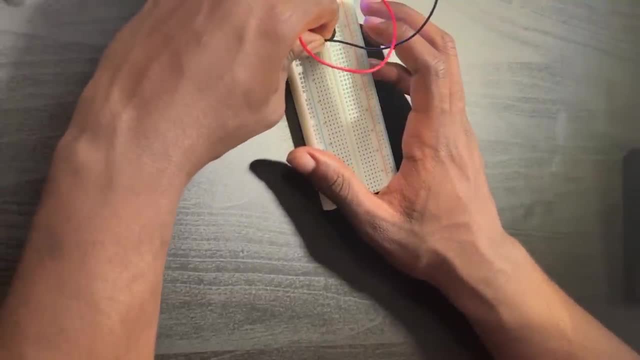 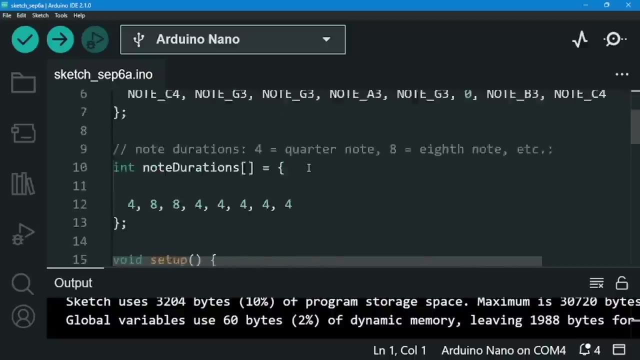 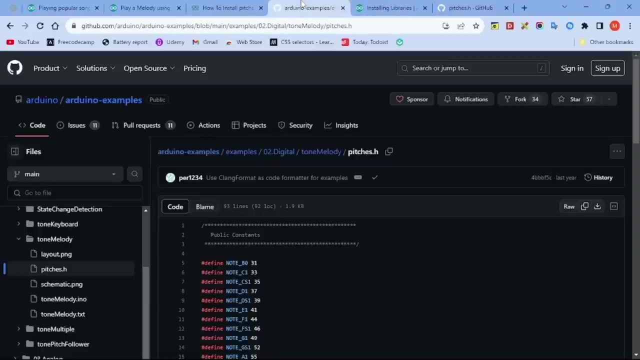 still getting the same thing. all right, so we're still getting the same thing. what could possibly be right now? i was trying to find another code, because this one does not make any sense. it doesn't at least be important what the pictureshe said, so it should have been actually better. 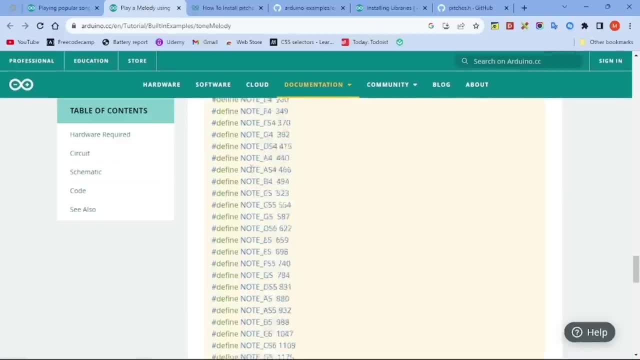 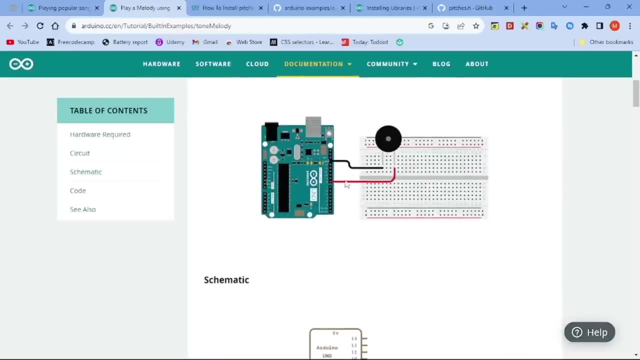 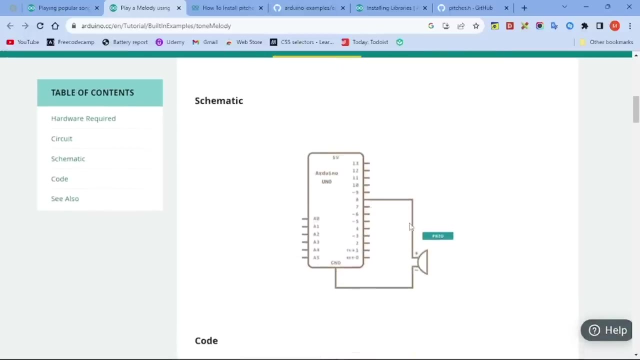 okay, so this one is horrible, or maybe i did not read one. i did not read the full documentation. what did it say? i have to connect it to what it specifically told me what to connect to. connected to what? pin 8. can you see that? specifically told me to connect to what to pin 8. 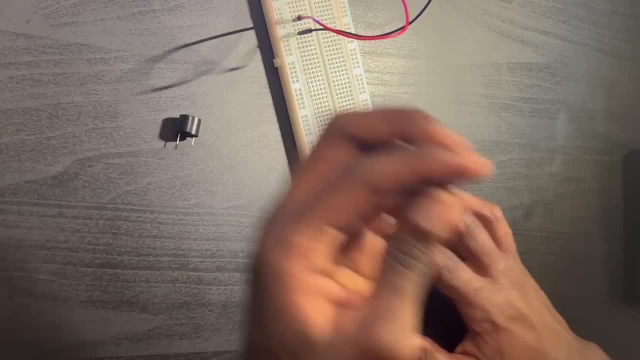 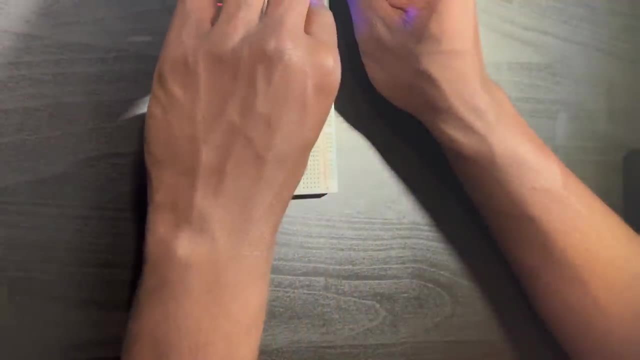 so I need to remove this active buzzer again. I did not read the whole thing. that's why I was rushing again to finish this video. that's my problem right now. but again it happens. I just wanted to show you guys. okay, actually I did not know anything about adding libraries towards. 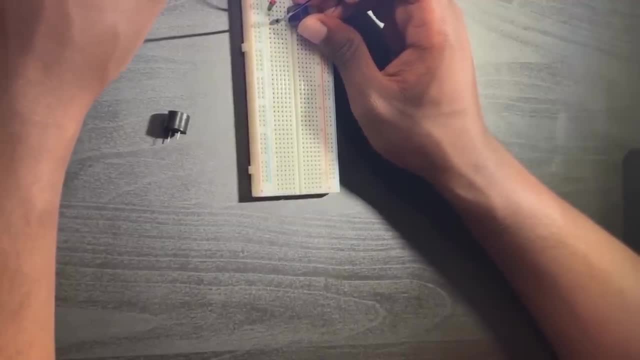 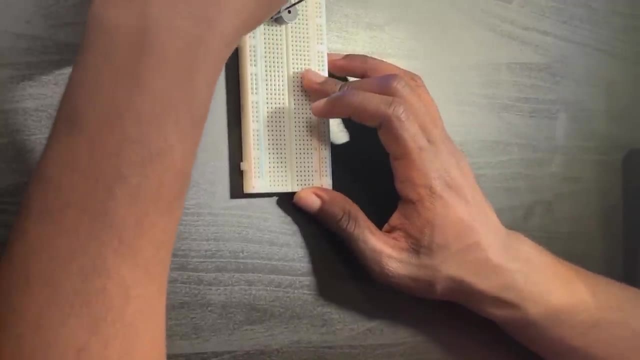 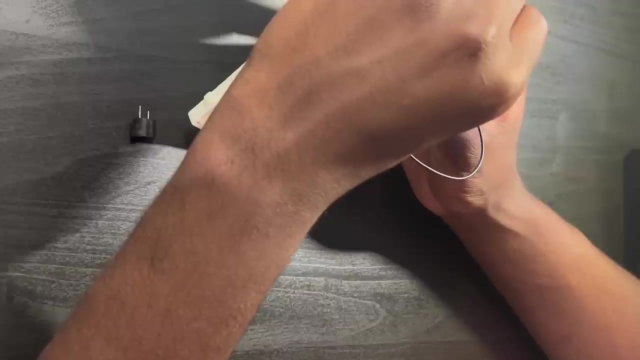 C++ or Arduino, but I just wanted to show you guys the process of learning. okay, me myself getting into a bit of a trouble right here. okay, so we need pin 8. it's hard to actually get the pin 8 right now when you're there's pin 8. all right, I think it's this one I'm supposed to be doing this. 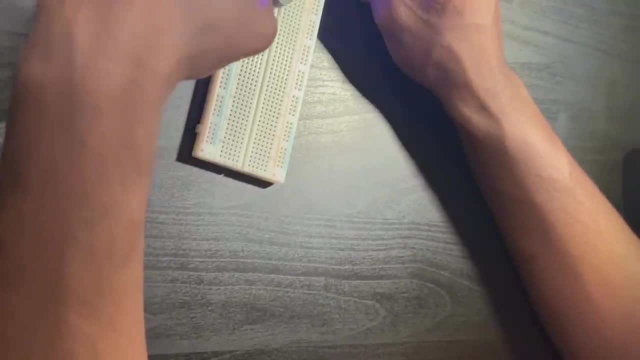 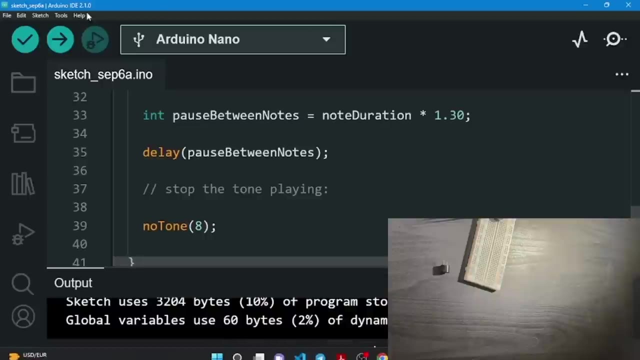 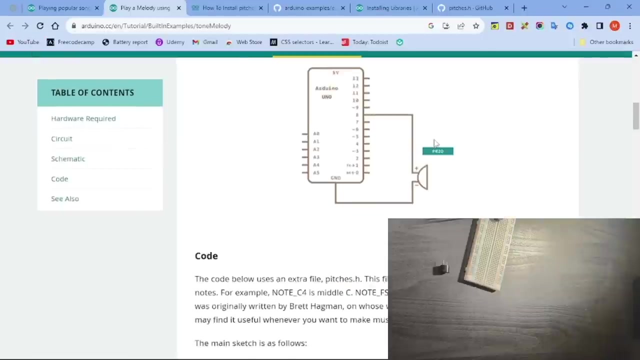 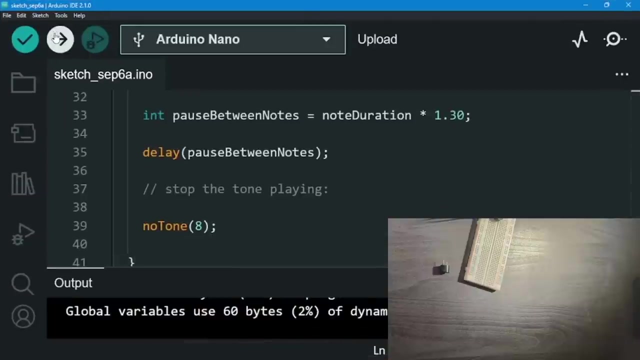 pin 8: all right, the gnd: uh, I uploaded it right. just make sure if I uploaded it or not. just to make sure right now. okay, it's done compiling, can you hear? let me stop for it again. okay, that's a nice tone right now. okay, how about I just want to run this again, and again, and again. 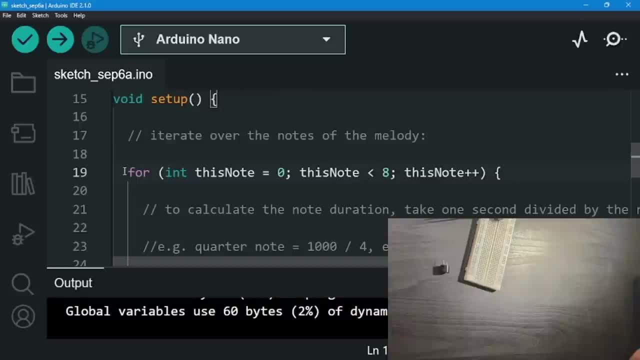 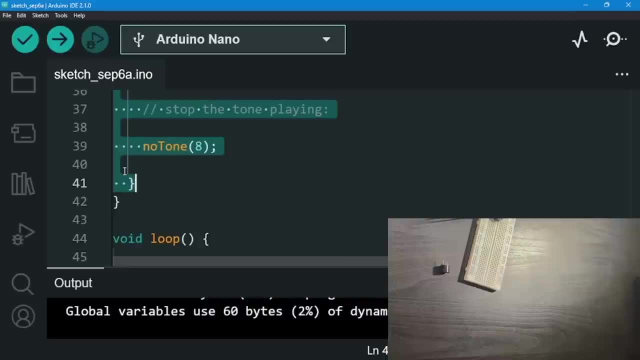 and again. it's just running one more time. what if I run this in the right here and just run it, set it in the loop, because I just want to run it again, again and again and again? that's what I want to do. want to run it on the loop right here. though, before uh finishing here, I'm just going to just 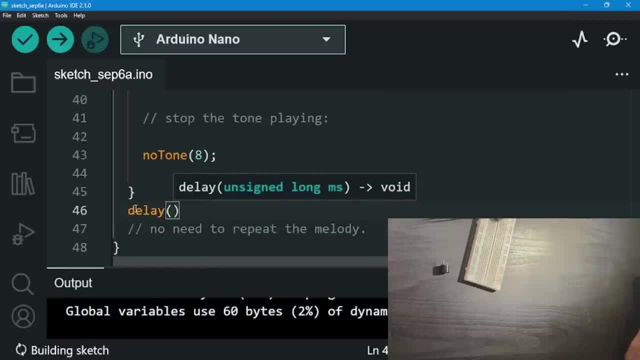 give it a delay. before you know, writing the tone over and over again, I'm just going to get a delay for maybe 10 milliseconds and it's going to make it better. I don't know if it's going to ruin the code. we're just going to see right now. 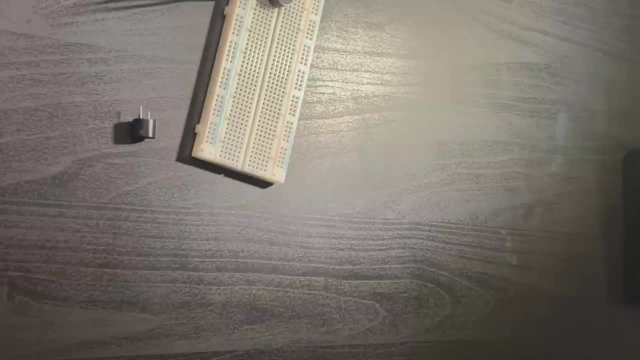 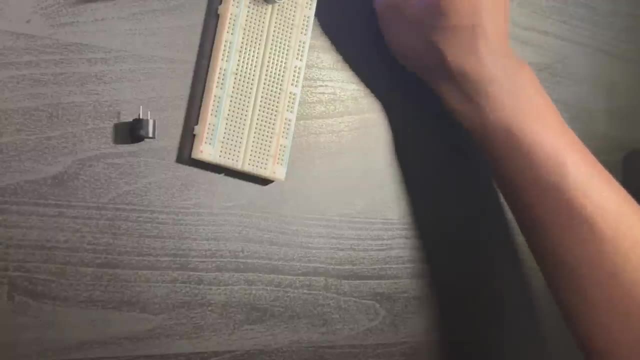 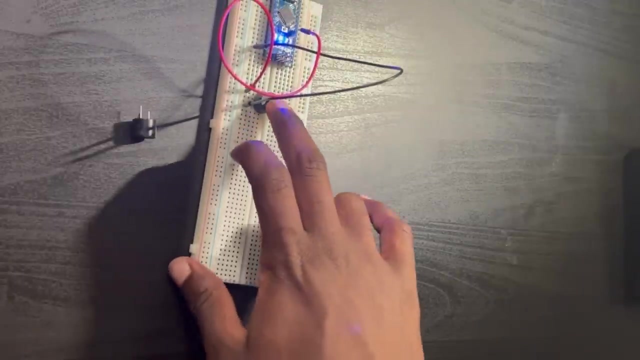 all right, all right. so this was a bit of a long one. right now I don't think you can see the buzzer right here because, again, I just moved it around, but I don't think it matters. again, I just connected it to what pin 8 right here. 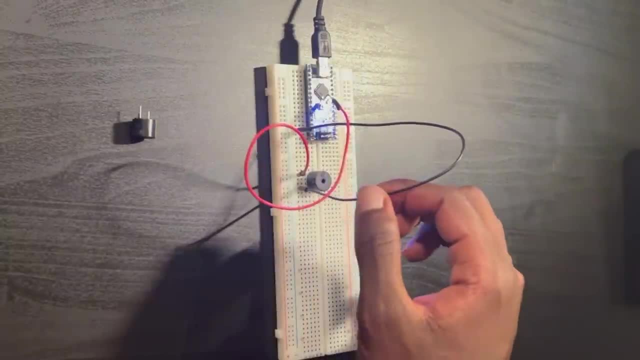 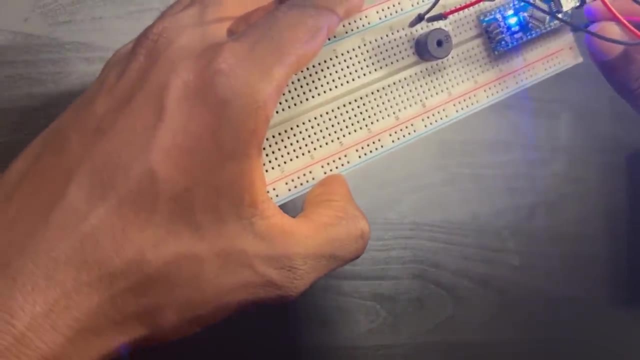 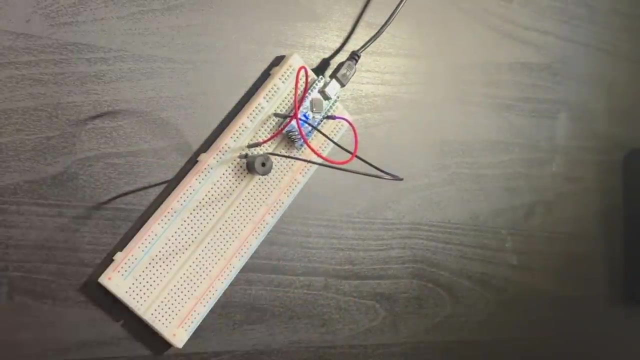 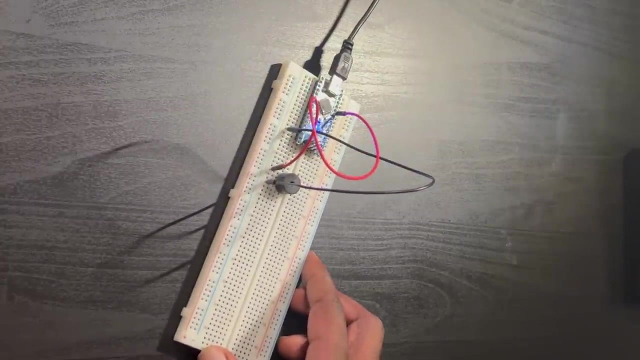 okay, connect this one to pin 8, and I connected this one to what the gnd? that's all I did. this is what to pin eight, as in the image, is connected to what to pin eight. it's just my uh, it's because that my uh, my wire isn't that long. here you go, you can hear it again. there we go. so i guess that's it. 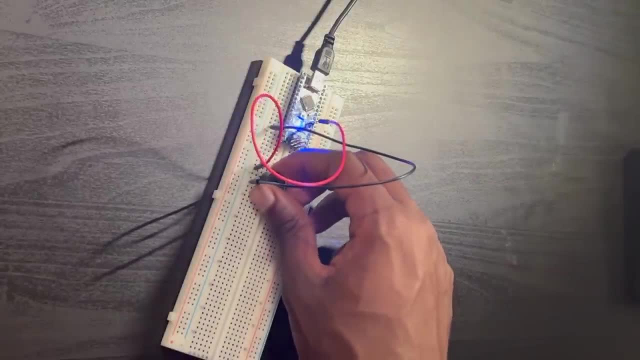 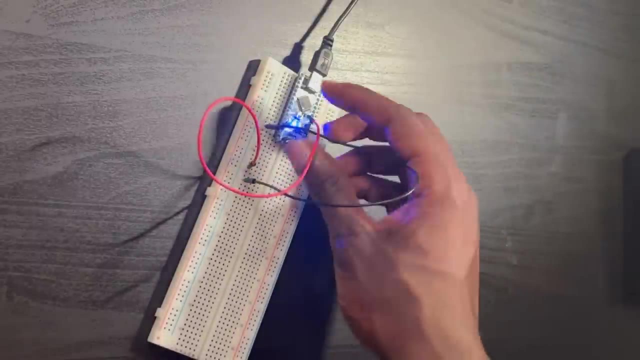 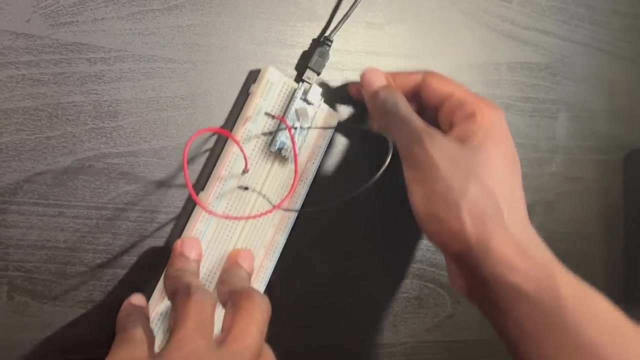 for uh today. uh, yeah, so actually see, on the next section. this was a bit of a long one and really sorry, by the way, for uh if you guys did not see the uh the pins. i tried to tell you guys where i connected it to and all. but again this just happened because again my wire isn't that long. 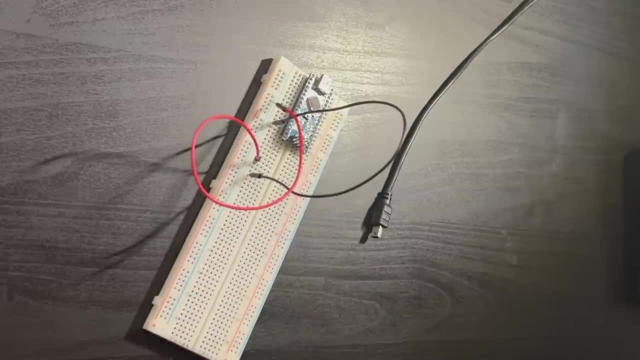 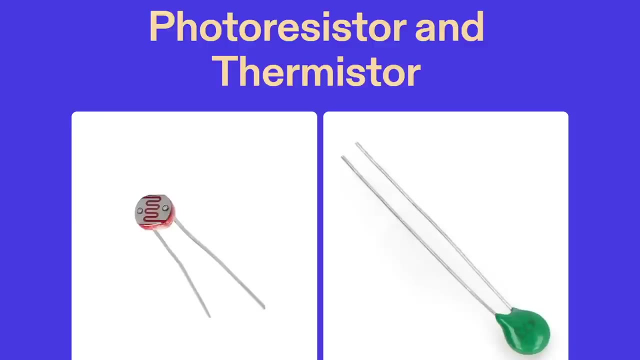 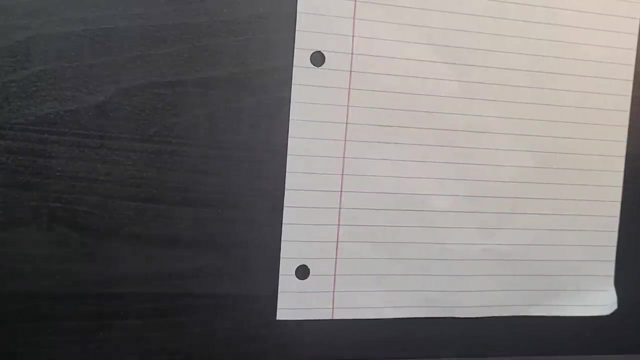 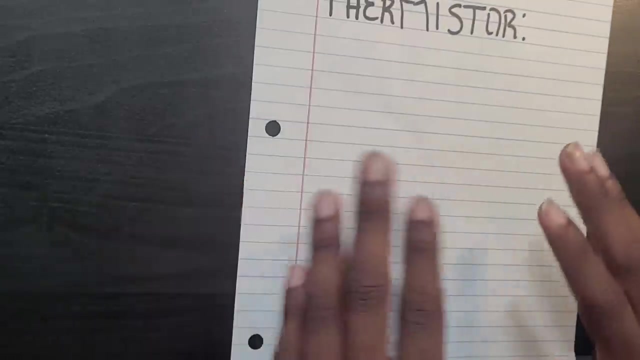 and i have to pull it really hard to actually bring it here. okay, anyways, see you in the next section. so here we go. okay, so in this section we're going to discuss about, uh, photo resistors and termisters. okay, so let's bring something that is familiar with you guys: resistors. obviously we use them to do. 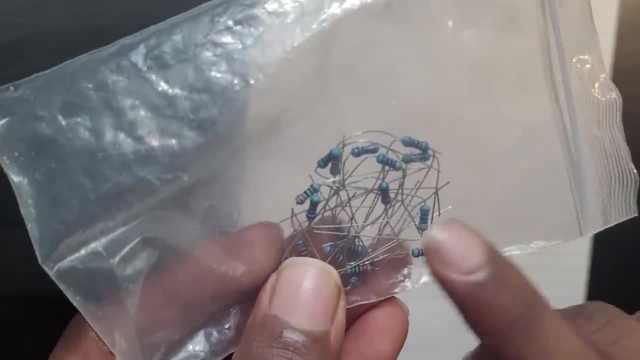 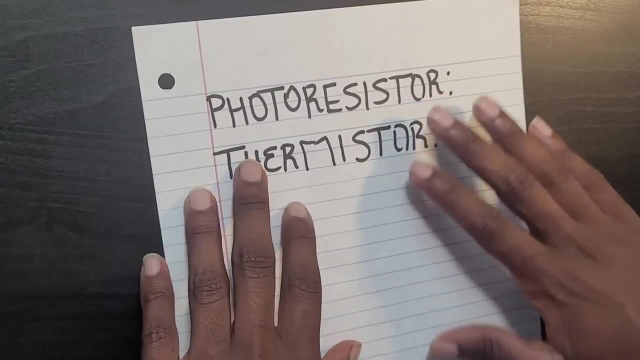 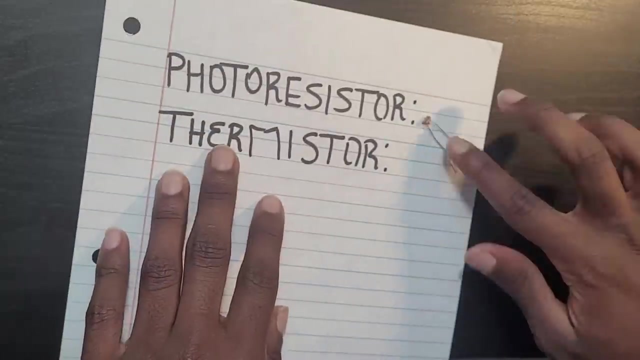 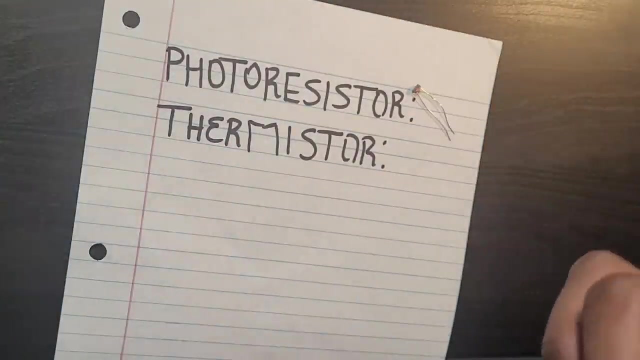 what to limit the amount of current that is coming in so that it does not basically what ruin our components. okay, so right here we're gonna learn about these special type of resistors, so let me just bring them right here. this is a photo resistor and a therme. therm resistor looks something like this: 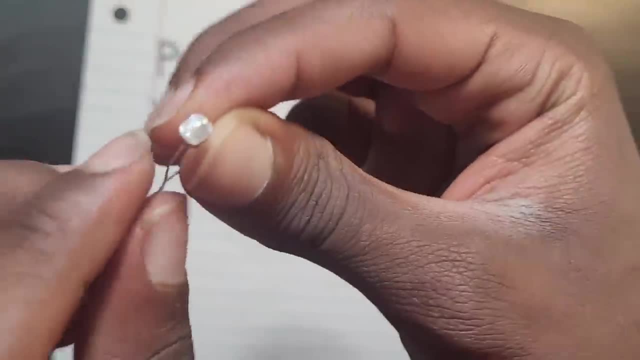 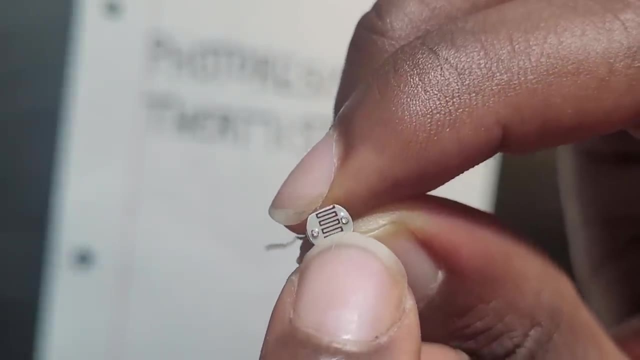 let me bring this close enough so that you can see see them for yourself. so when you're looking for a photo photo resistor, what you're going to be looking for is this quickly lens right here that goes like this, like this, like this. okay, i'm going to be looking for those. 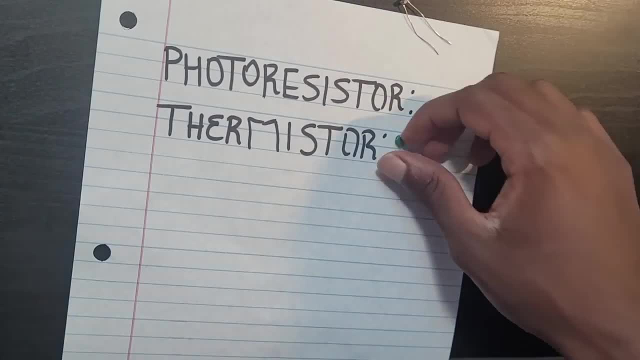 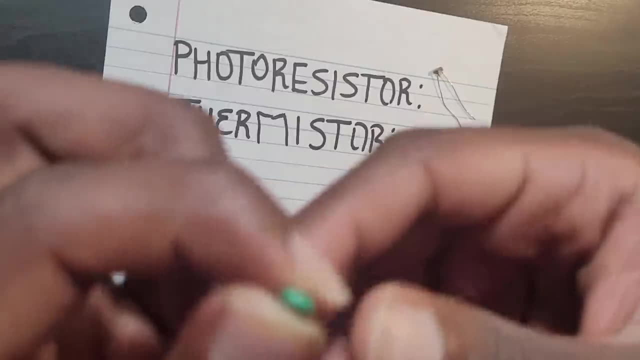 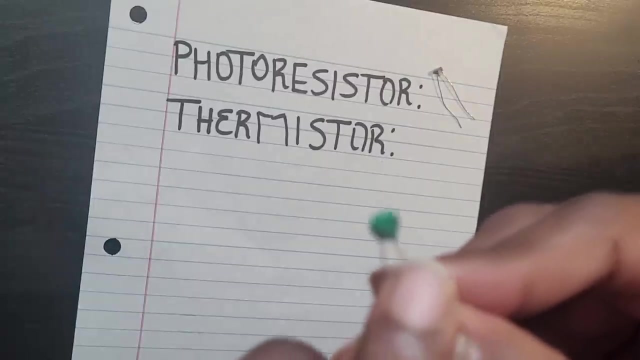 when you're looking for a photoresistor- and let me just put that next to its name- and when you're looking for a therm resistor, you're going to be looking for these round headed again. they can be green, they can come in black, but again, always read your labels to make sure what you have right here. 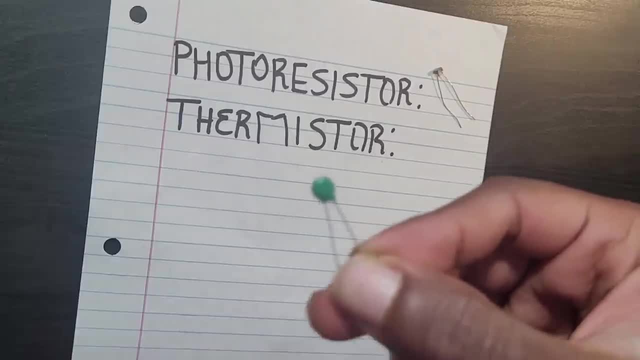 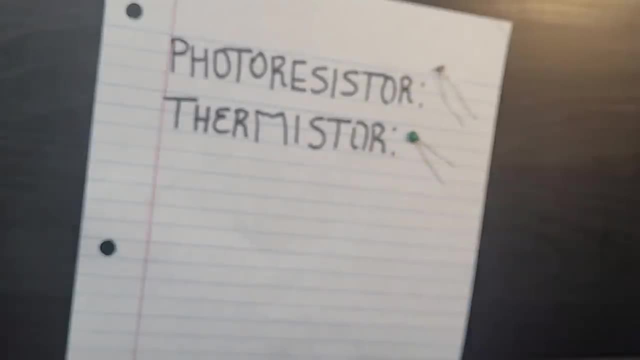 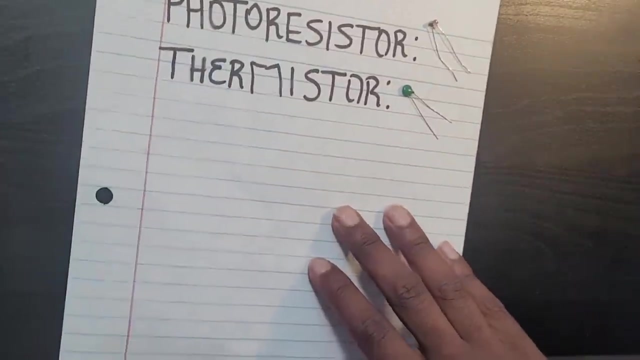 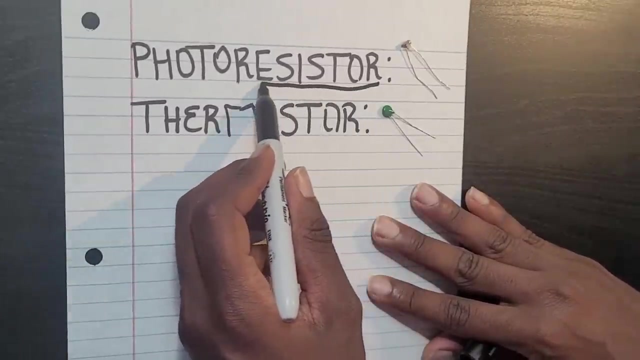 okay, so always make sure because they look close to something called ceramic capacitors. okay, so just keep that in mind. let me just put this back to its place. okay, now let me try to explain what these are. okay, so these are, as I said again, they're types of what resistors there's some. 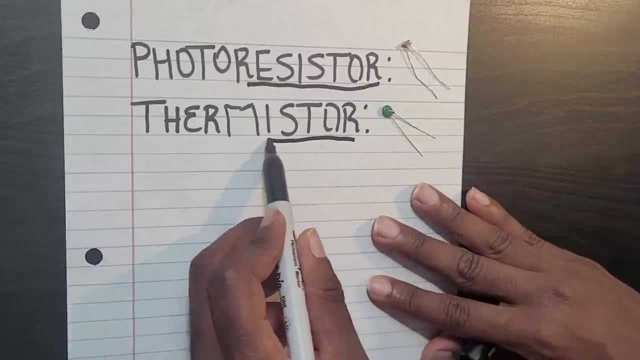 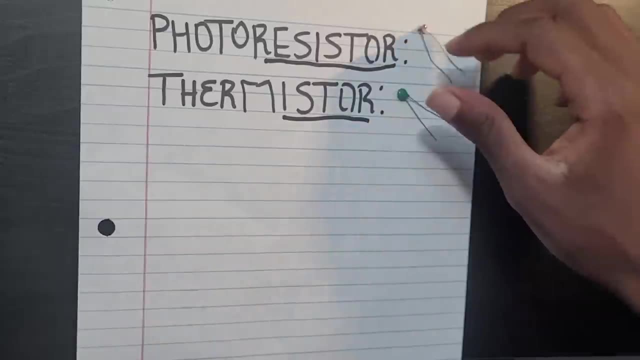 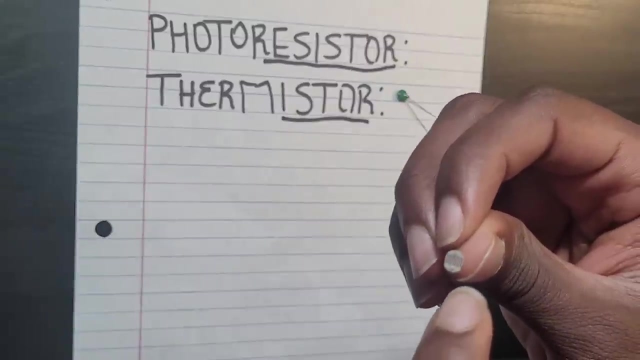 sort of type of resistors. they have the ending of ister, okay, so there are different types of resistors. so, when it comes to the photoresistor, when it comes to the photoresistor, one thing you need to understand is it is a type of resistor where the resistance value changes- okay, depending on light, obviously. 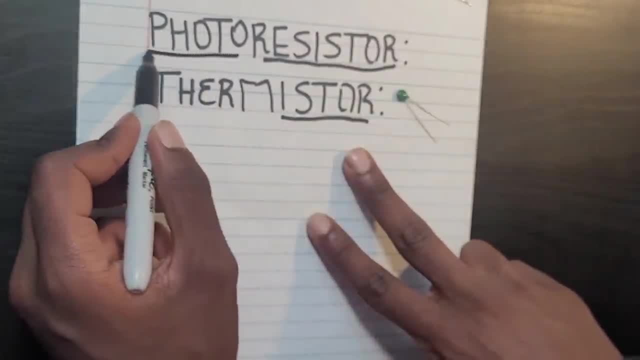 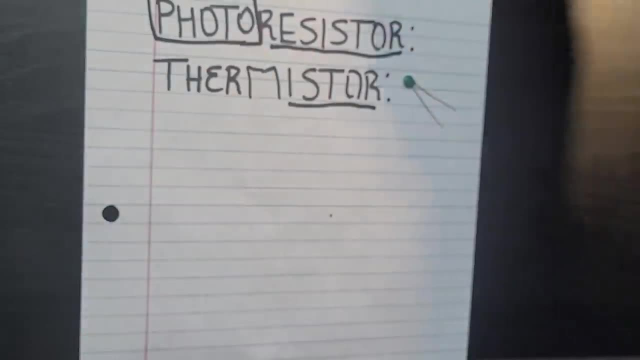 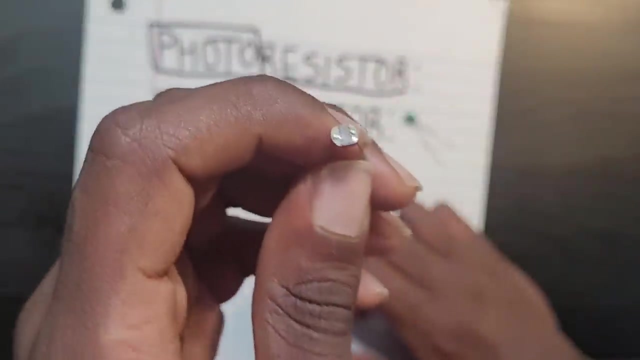 the name photo. the beginning of photo indicates something that has to do with what with light. just like how we use photosynthesis has to do something with what with what with the light. so photoresistors are what these are: types of resistors in which the resistance value changes. 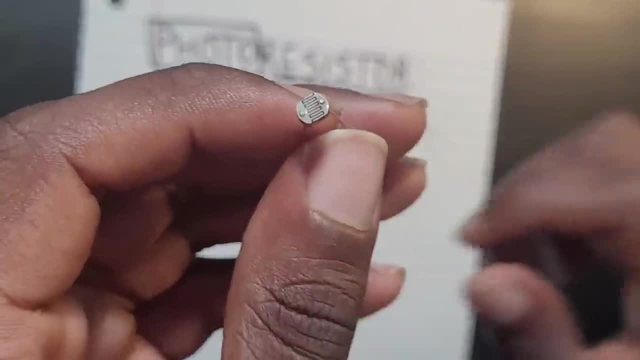 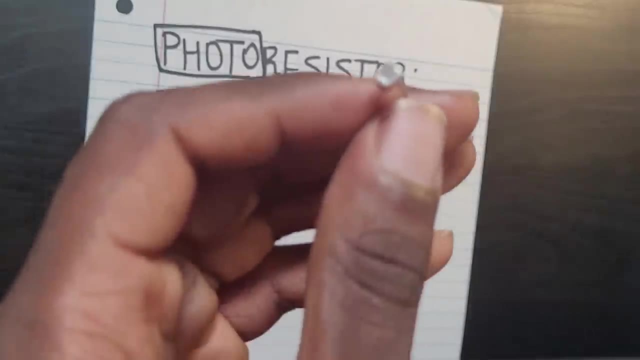 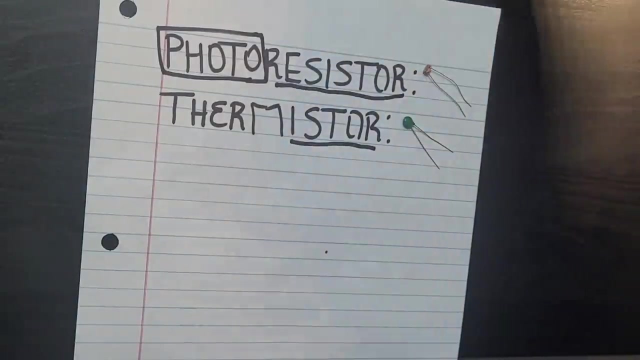 according to light. this happens so that because we use a, a special material, all right, on the top, we use a special material which changes this resistance again corresponding to what corresponding to light, all right. so one good analogy of this would be something we've worked with in the previous project, which is going to be- uh. 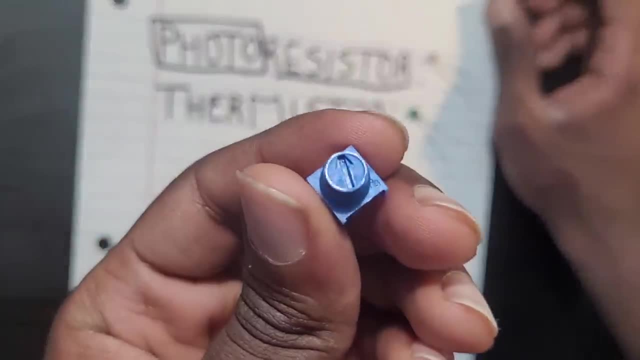 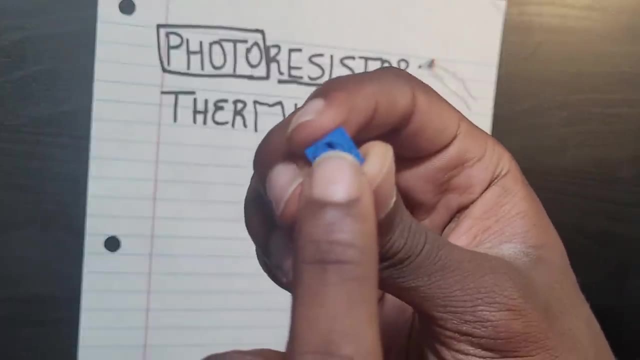 it's going to be a potentiometer right here, let me just bring it closer. the potentiometer we just worked in the past few sections. so, potential meter, what happens? how do we change its resistance? it's a variable resistor, as i said again, how do we change the? 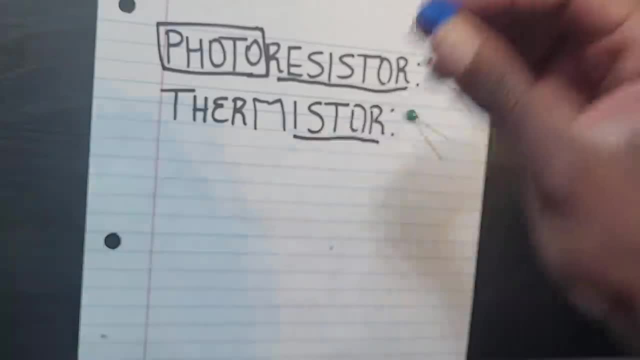 resistance. we just change the knob, just like this. and when it comes to a photoresistor, what do we do? we change the light, we change the value of light, so we change the light again. we go dimmer and brighter and it's going to change our what, our resistance? okay, just keep that in mind, all right. 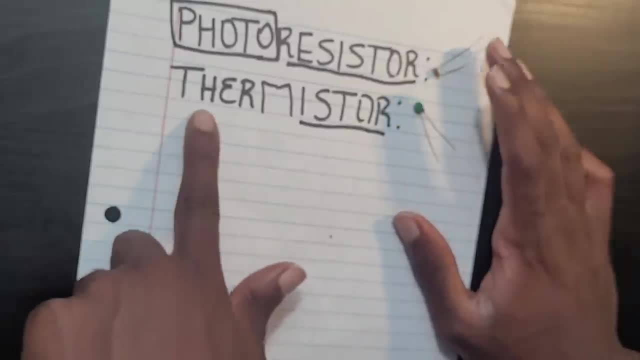 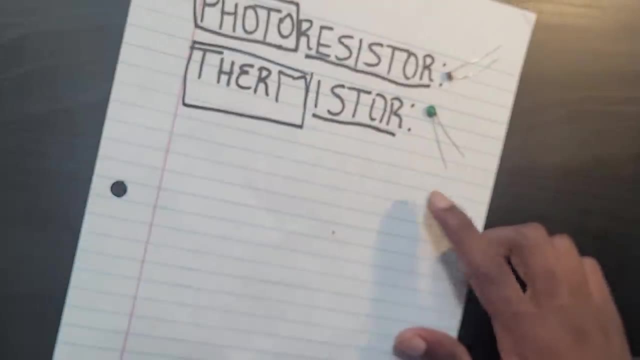 when it comes to our therm resistors. the name thermy gives it away. this is related to what? something that has to do with what? with temperature. okay, something that has to do with what, the temperature. so, when it comes to therm resistors, basically just like how photoresistors again. 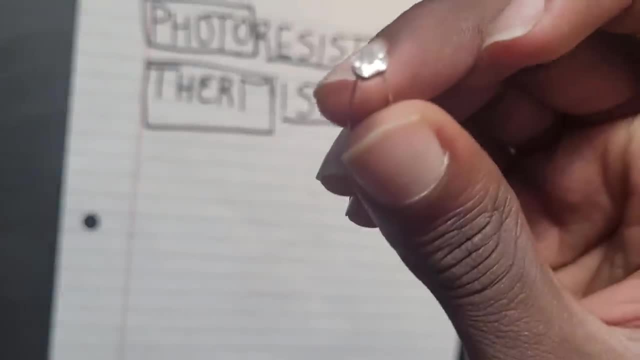 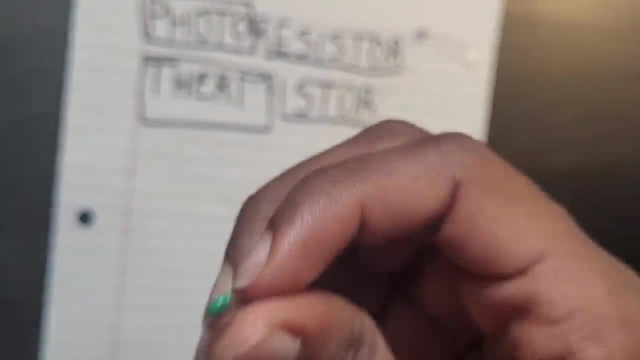 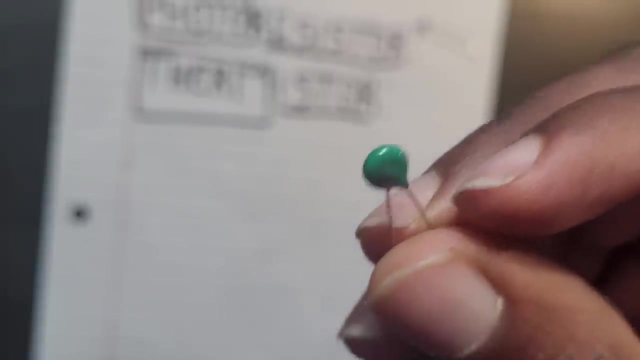 change their resistance value according to what according to light, just like a full resist changed their value according to light. these therm resistors, let me just go closer again. these therm resistors change their value according to what according to temperature. okay, according to what according to temperature. just keep that bold in mind. okay, so now i start, i think, uh, working with. 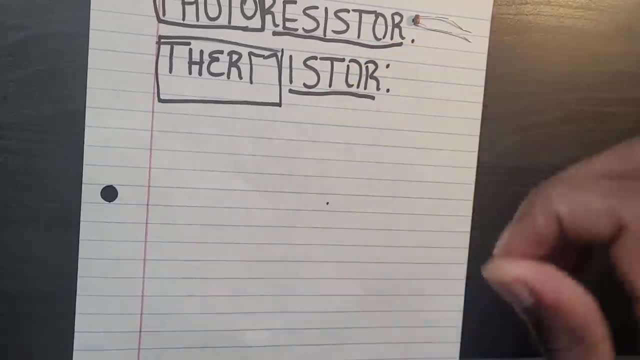 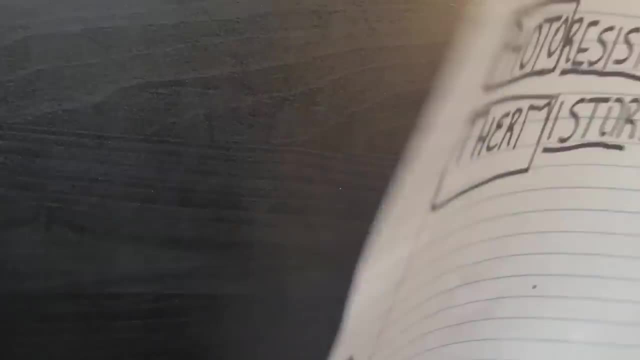 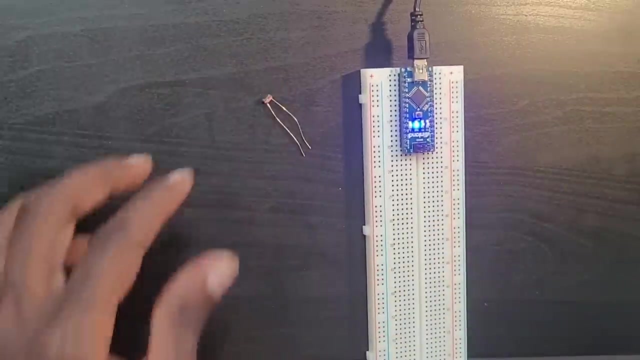 here. let's just keep our term resistor on the side here, because they're very familiar. that's why i just chose to teach them together, but let's work with our photo resistor first. okay, so let me just get this out of the way. just bring my arduino here. i have my photo resistor and what i'm going? 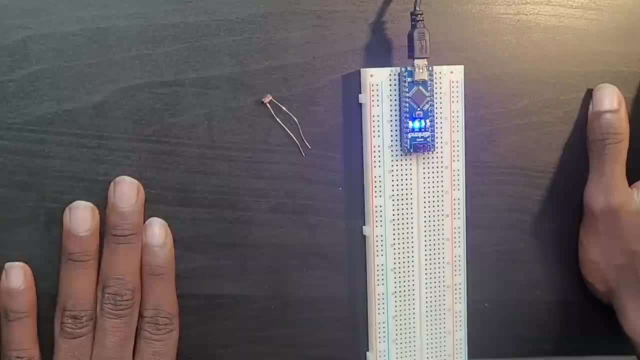 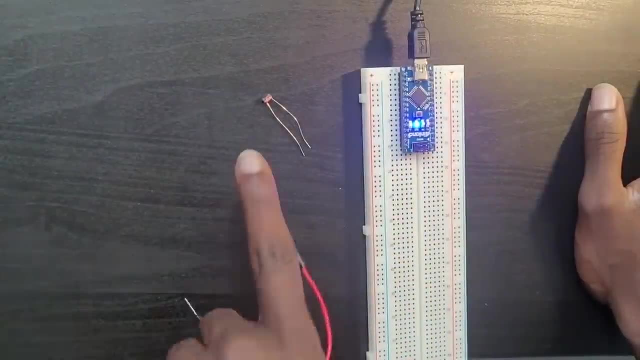 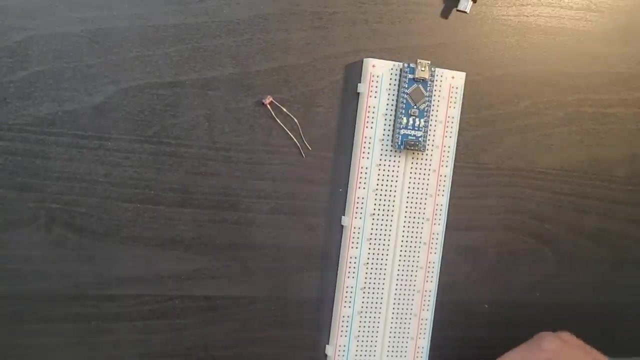 to do is basically connect a simple five volt circuit. so, just how we used to use an led in the resistor, instead of using a resistor, we're going to be using what we're going to be using: a photo resistor this time. okay, let me just turn off my light here. let me just turn it off. turn off my. 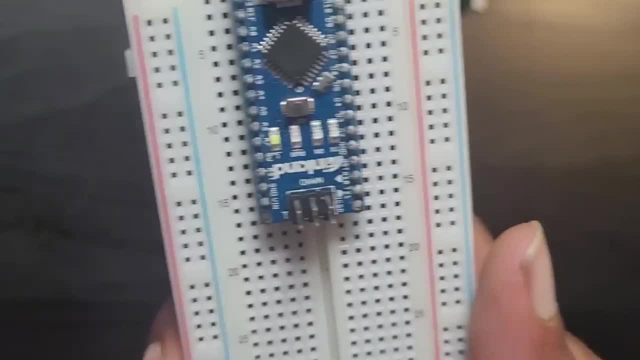 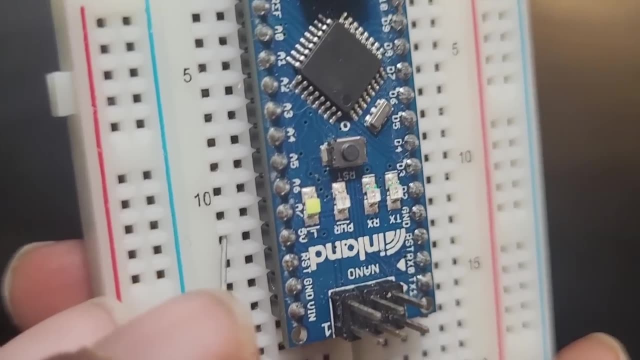 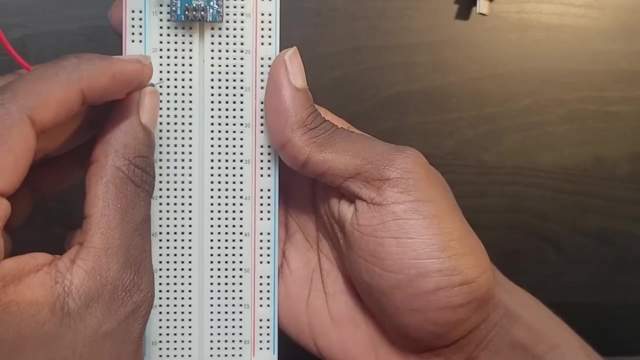 arduino. bring the arduino closer so we can focus on what we're doing right now. okay, there we go. i'm going to connect the 5p right here, the 5 volt connected to the 5 volt pin, the red, the red wire, right. nice. now what am i going to do? i'm going to bring it here, move it to here. 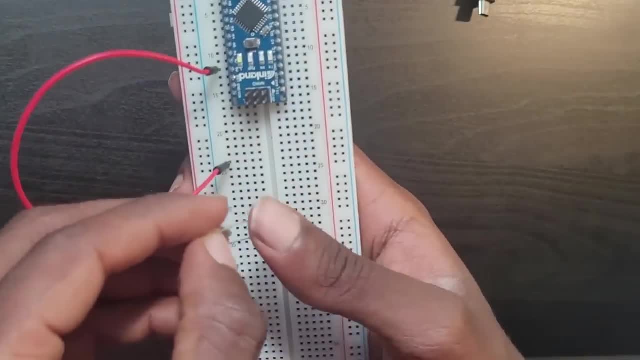 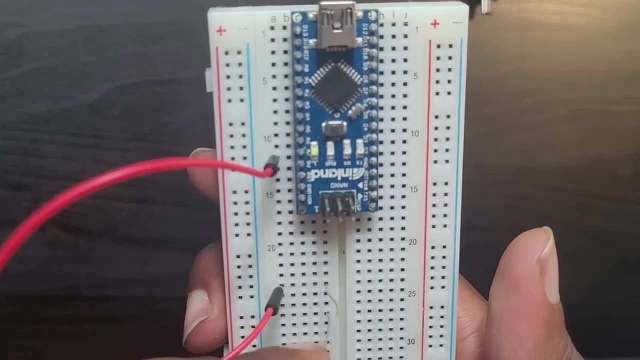 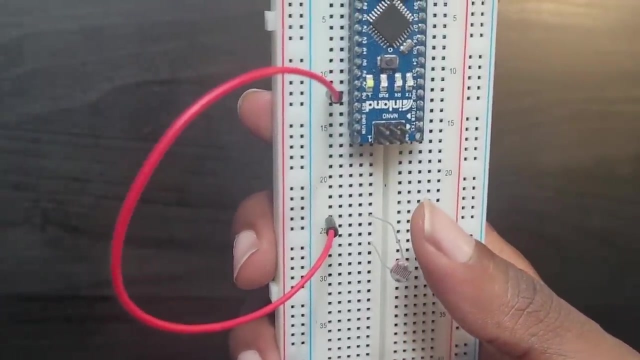 okay, then i'm going to have my resistance again here. i'm going to put it across. okay, when it comes to resistance, again, it does not matter which leg you put it through. obviously this matters in leds, but when it comes to any type of resistance, it doesn't matter which leg you put through first. okay, the same comes to. 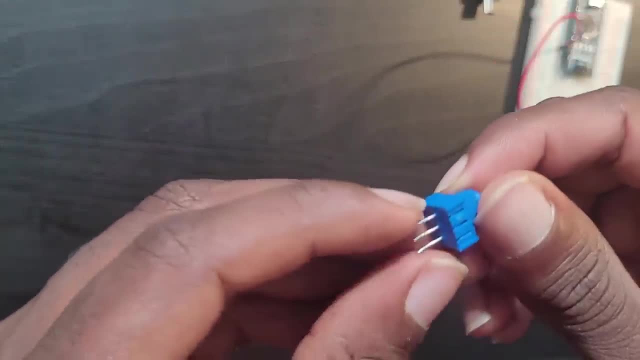 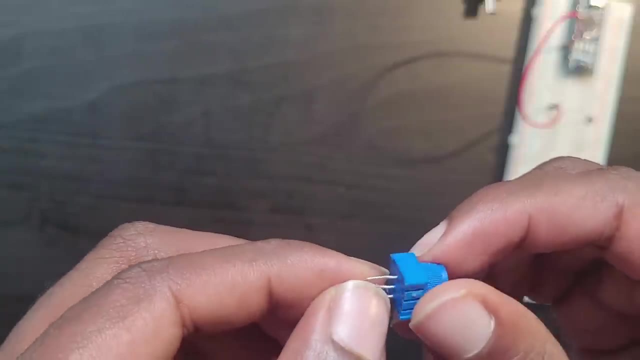 potential, the potential meters. you can put what- the first leg or the last leg, it doesn't really matter. what matters is the middle leg. obviously it's going to be the one with the v out. so obviously the middle leg is the important one. so i'm going to put it here and then i'm going to 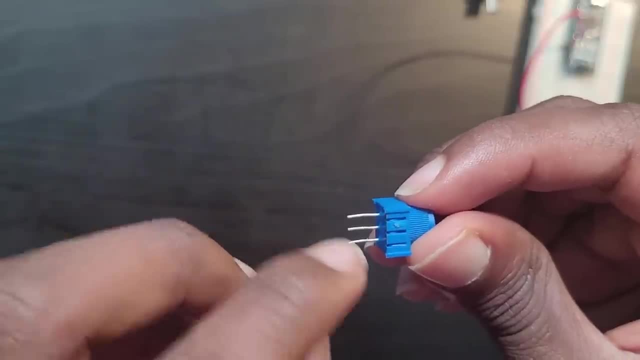 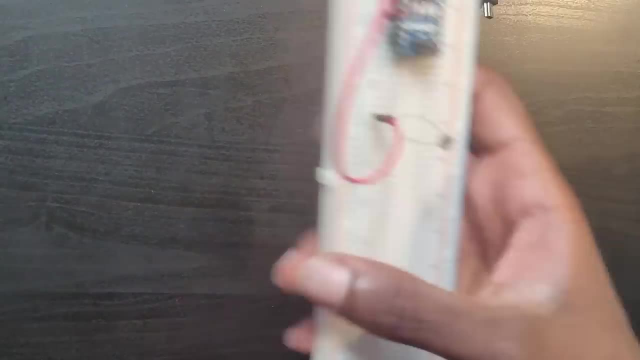 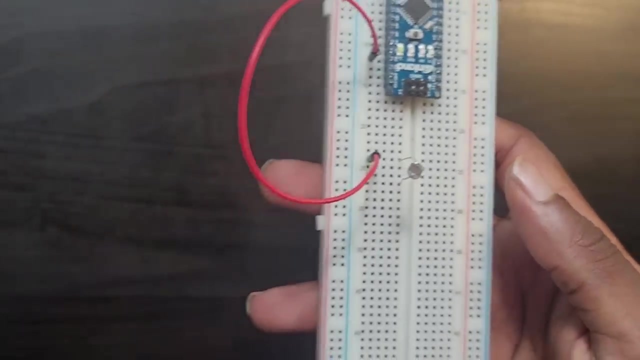 connect the other one that you actually don't want to mess up. but you can just choose between these two. you can just put it in the gnd or this other side on the 5 volt, doesn't really matter. okay, let me just put that here, focus on it again. all right, let me get my led, my handy led, right. 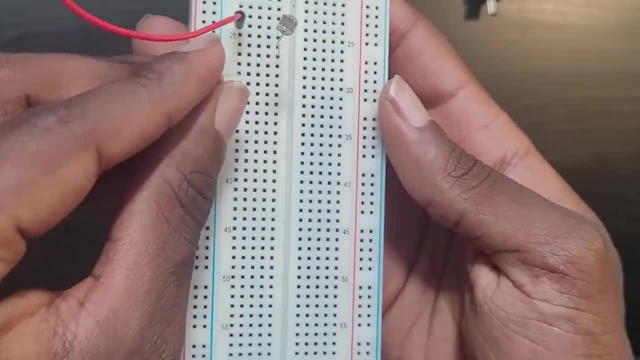 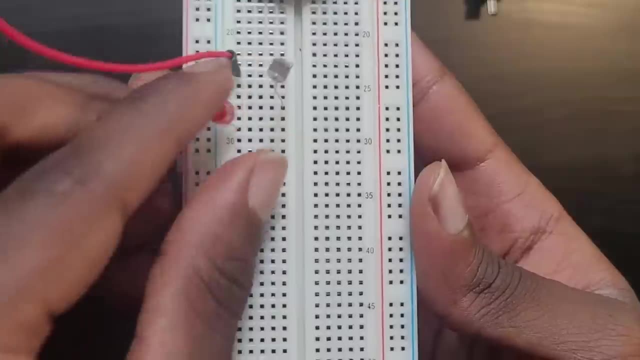 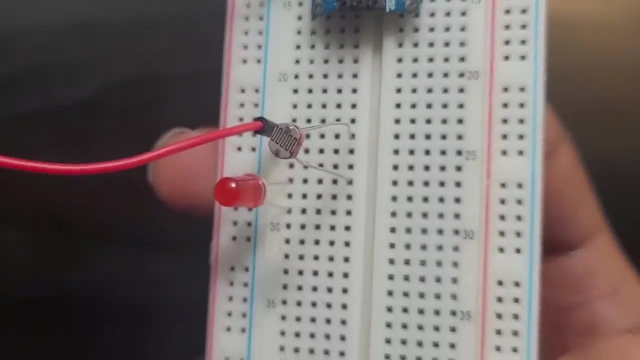 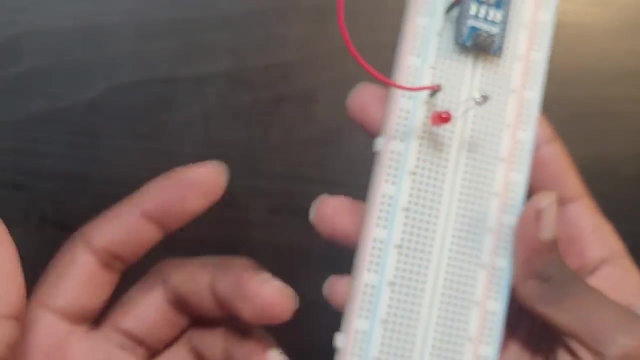 here, got my led. now i'm going to connect one leg of the water resistor here to the what to the led. let me just do that, just focus here so you can see it better. there we go now. you can see it way better. all right, and then what do i need? my gnd. 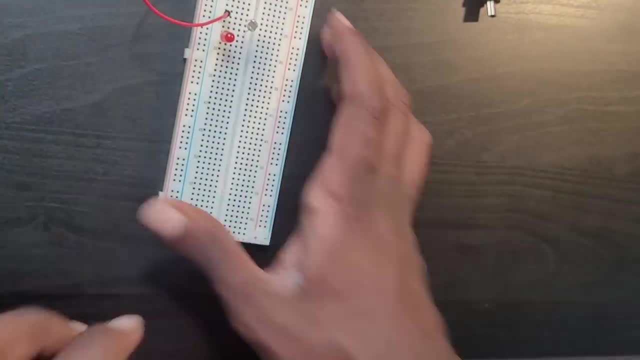 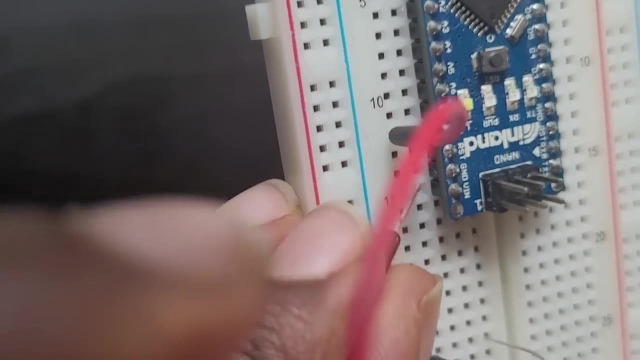 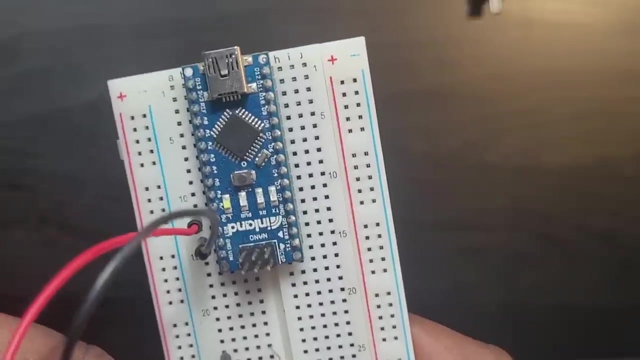 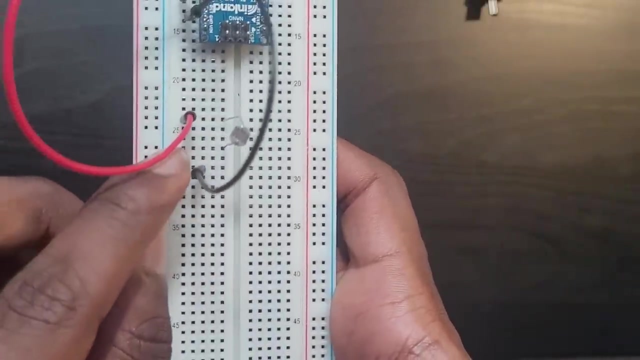 okay, let's bring the black wire here again, connect this to the gnd. where's the gnd? yet it's right here. i just connected the gnd pin or the negative terminal. let me bring this across here. great, let's just put it back here, to the other side of the what the led. 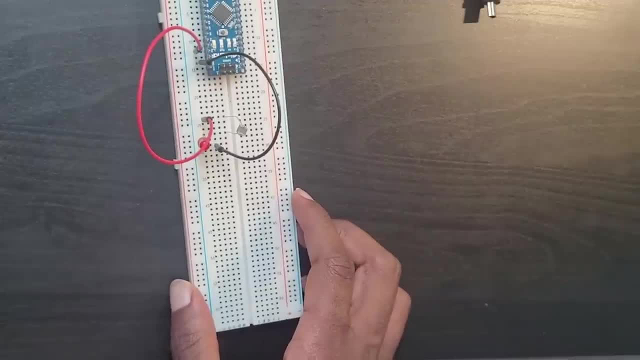 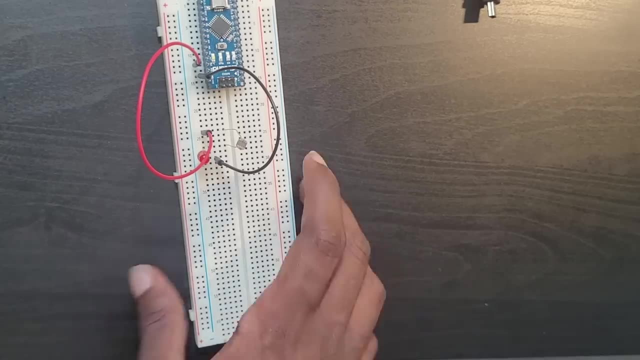 okay, we just did that. okay, we just did that. but there's something wrong with this circuit. i mean, it seems fine when you look at it, because, as far as i'm concerned, what did we do? let's just recap on it. what did we do? we used our. 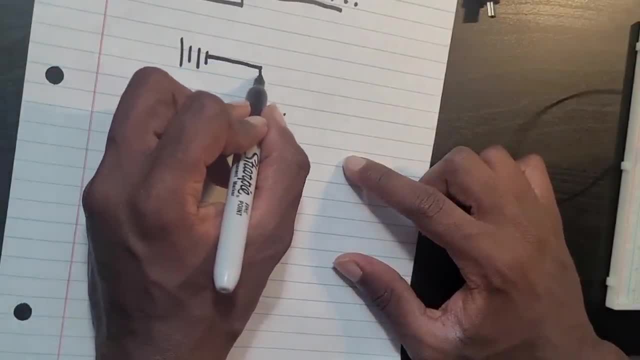 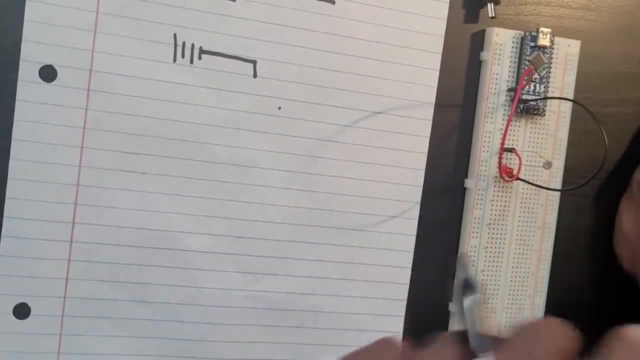 you know as a five volt output, because we connected the what to the five volt. and then, what else did we do afterwards? we went to our what- let me just bring this aside here. what did we do? we brought our resistor here. in this case it's a variable resistor, and you just 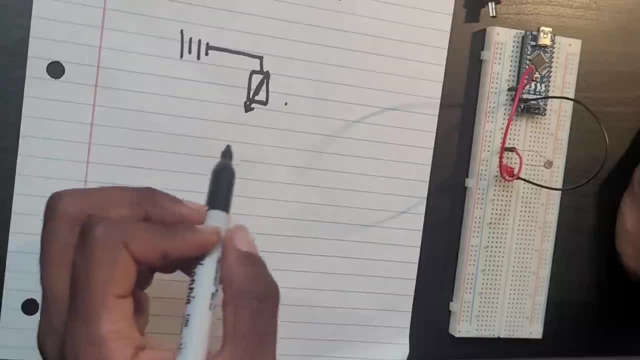 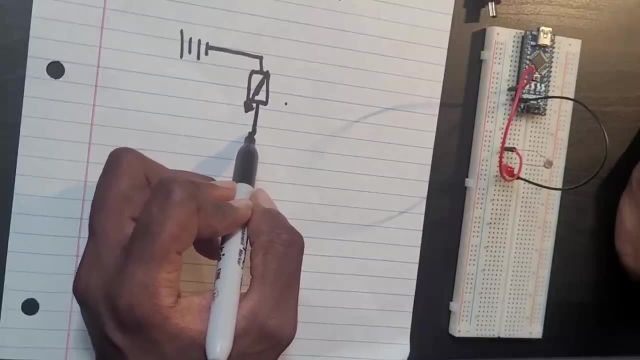 indicated by this, by this symbol. variable resistors indicated by this symbol basically changes what it's resistors, it's resistors values. this value changes according to the condition. okay, in this case, what it's going to be, the condition is going to be the value of the resistor. 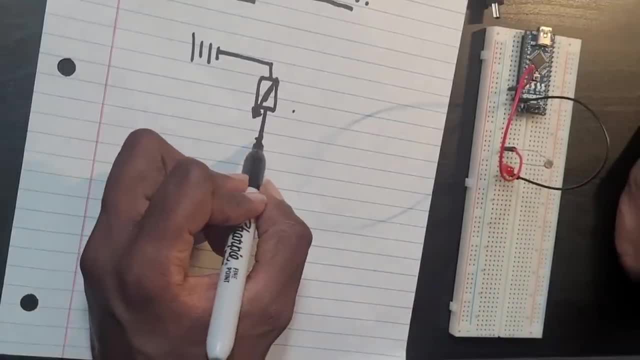 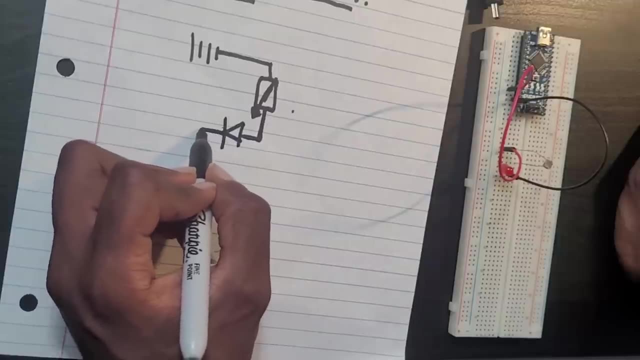 okay, in this case, what it's going to be the condition is going to be the value of the resistor of light. all right, then we have our led, our handy led. how do we write that down? we go like this. then we go back to our negative terminal. 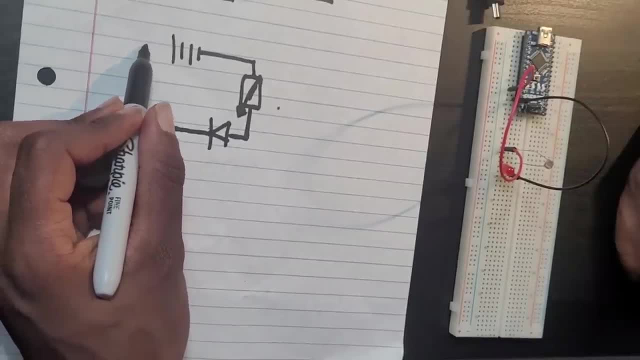 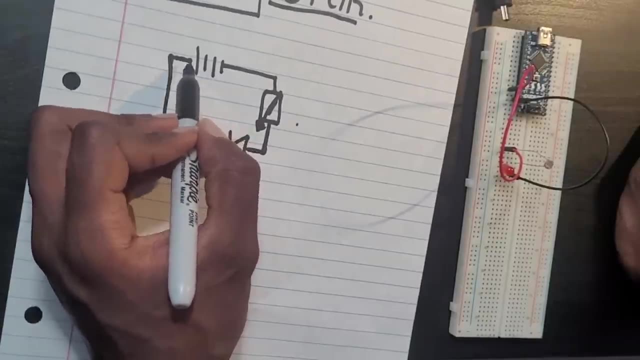 one thing i did wrong here is what this is the negative terminal. the negative terminal is what this the smallest side. so i have to put a negative here and have to make this the positive. i have to make it the bigger one because obviously i'm going to have to make this the positive one. 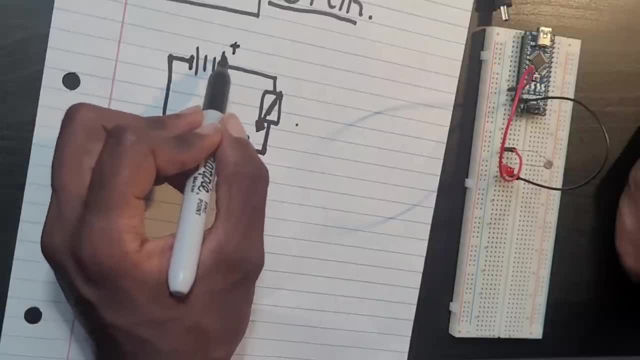 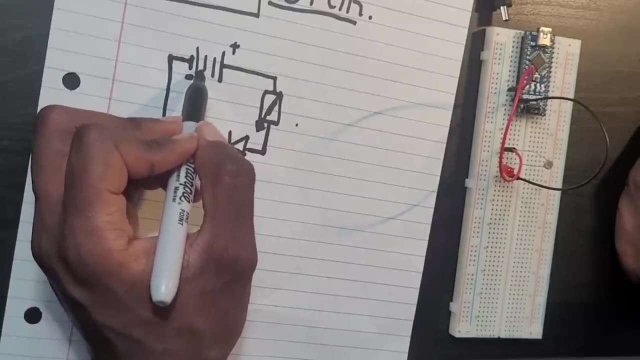 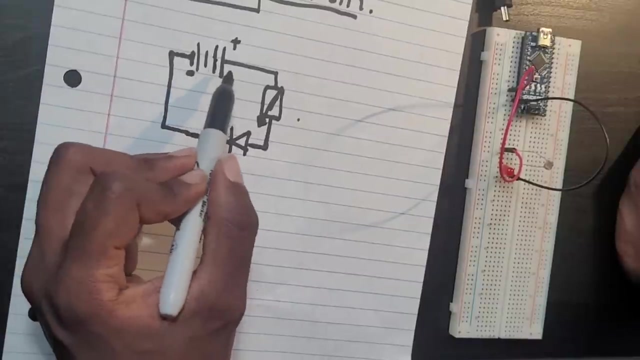 obviously why? because that the big one is the positive, the bigger line and the smaller line is what negative. okay, let me just put that. and again, let me just correct this: this goes big, small and there's a small one. all right, there we go. i'm just correcting this, anyways, what basically happens? 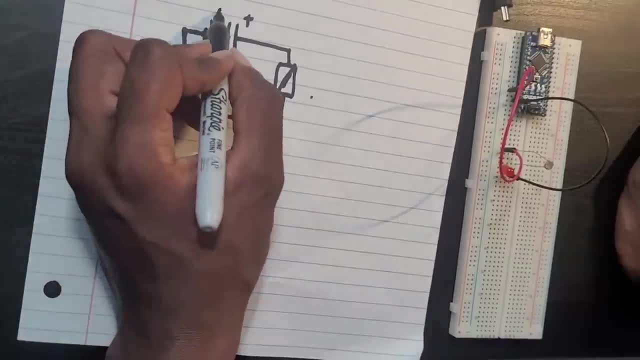 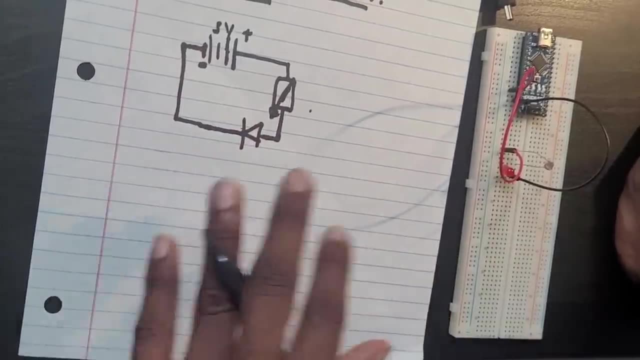 here is what we have: the five volt output. we have our resistor, we have our led. this seems like a normal, you know, a simple five volt circuit. so we're going to have a resistor and we're going to get again. this should be working and there's nothing wrong with it as far as i'm concerned. 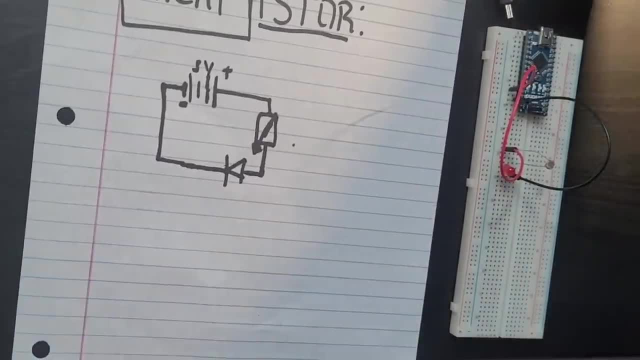 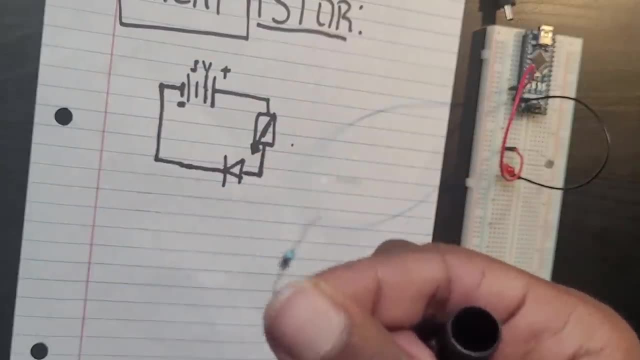 it looks perfectly neat. instead of using our normal resistor, right here, we just used some sort of resistance. instead of using our normal resistor that we have here. instead of using that, we basically did what? instead of using our normal resistors, we basically used what? a photo resistor. 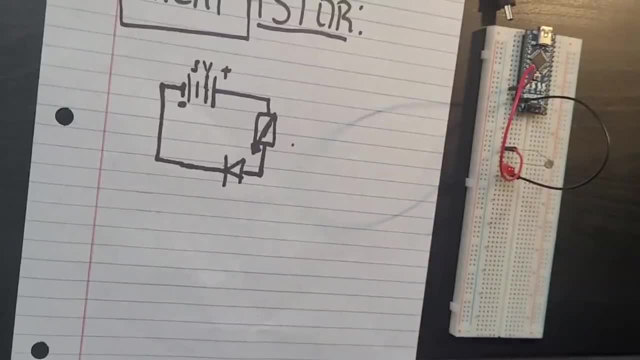 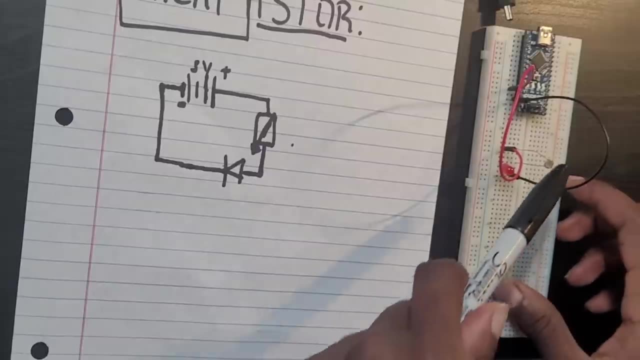 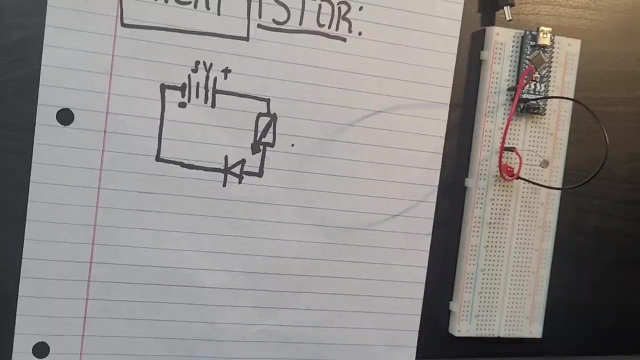 which we said is what it's a type of, what is a type of resistor. but the problem that lies here is that this photo resistor, the value changes over what? over light. so right here, i have a bright environment. all right, i have a bright environment, all right. so how am i supposed to be sure? how am i? 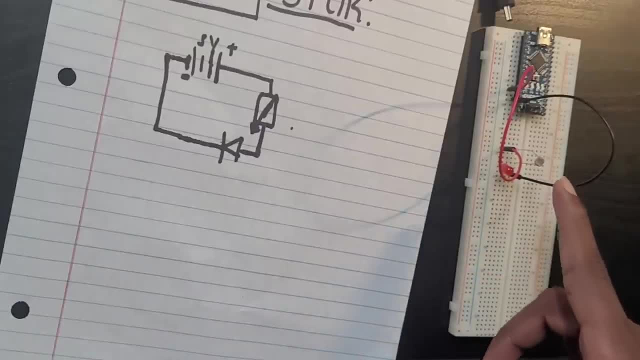 supposed to be reliant that the photo resistor, you know, doesn't have a small resistance value because, we said, the resistance value changes. how am i supposed to be sure that the resistance value is not very, very small? how am i supposed to be sure? right, because something you need to know about photo resistors right now is: as the light increases, okay, as the 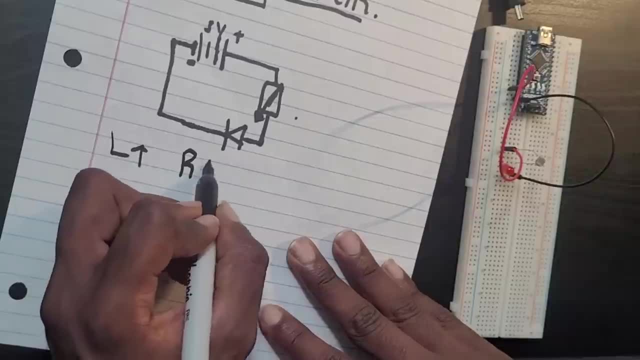 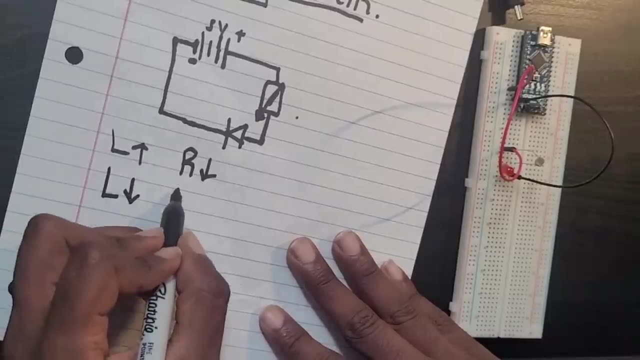 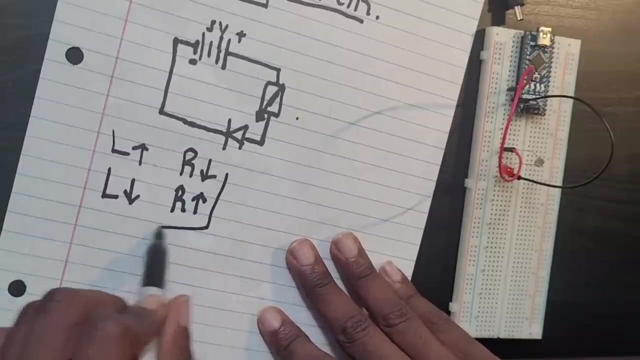 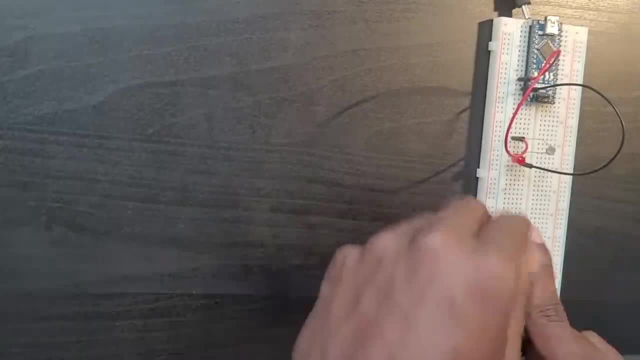 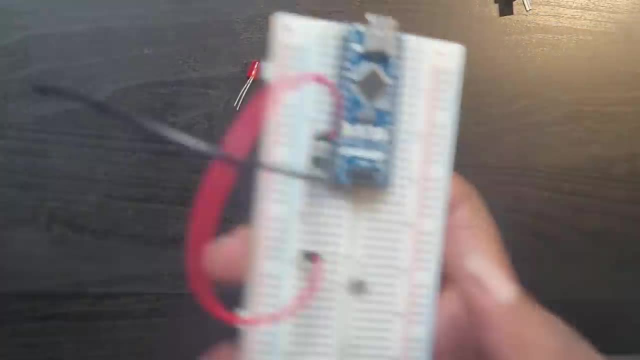 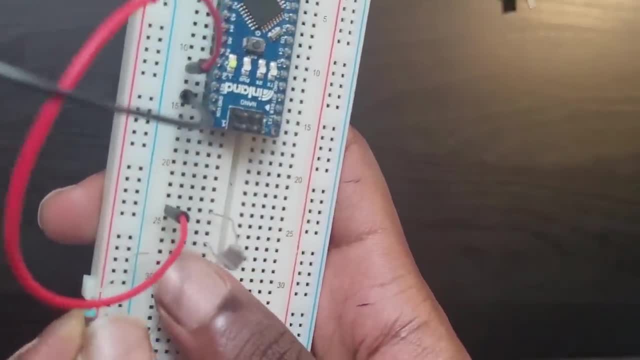 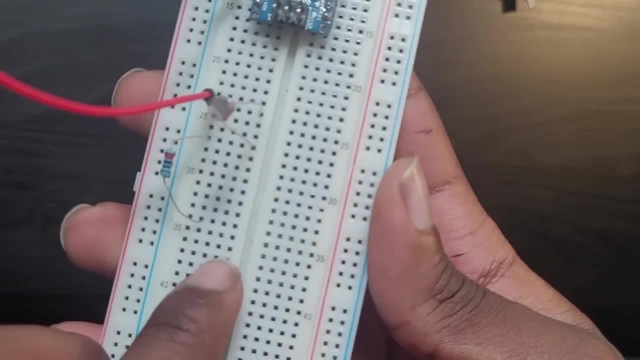 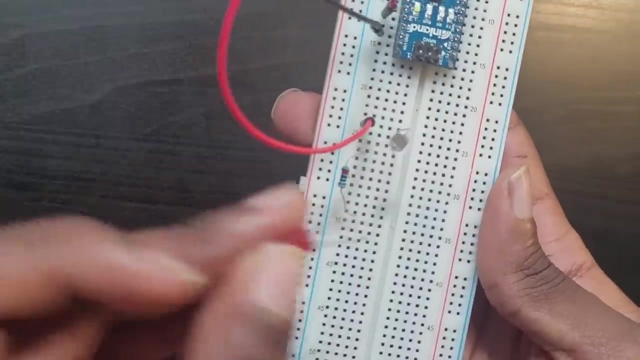 sorry photo resistor right here towards the other leg of the resistor, my normal resistor. all right, there we go. they're connected. okay, once i'm done connecting them, what do i need? i need my led again. always check for the positive side, the longer one, the longer side of it i found. 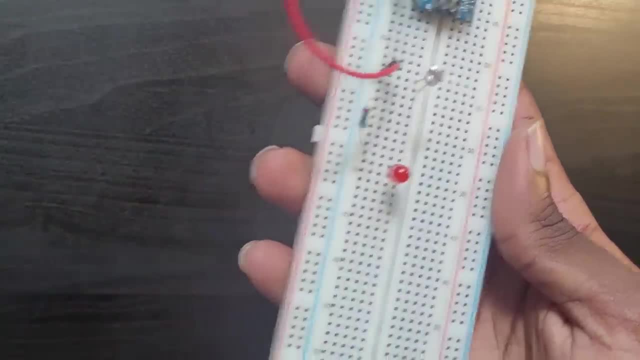 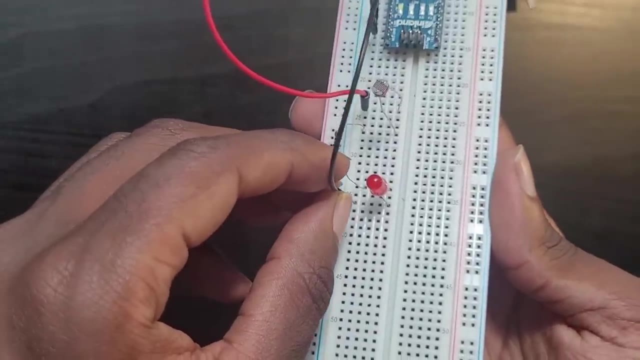 it. i'm just going to put it here, all right. and i'm going to need my what, my gnd pen. let me just use my what my gnd to the other side of the led. let me just use my gnd right here. all right now. 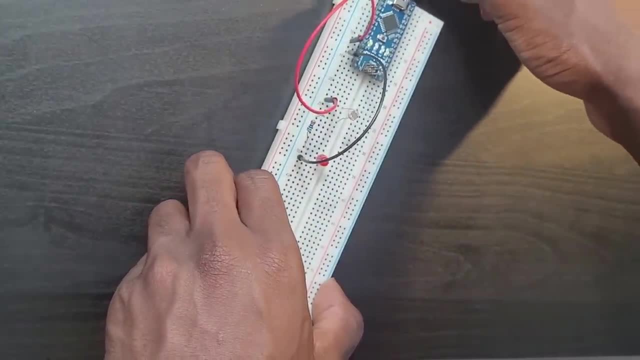 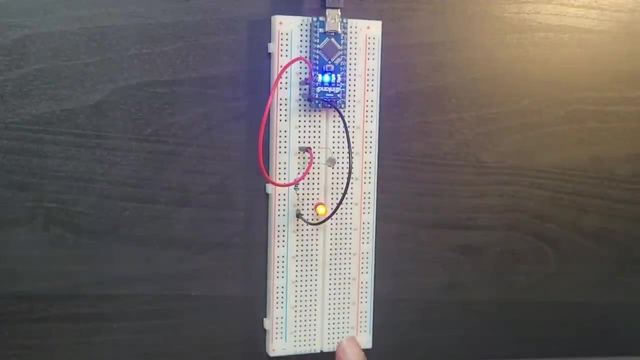 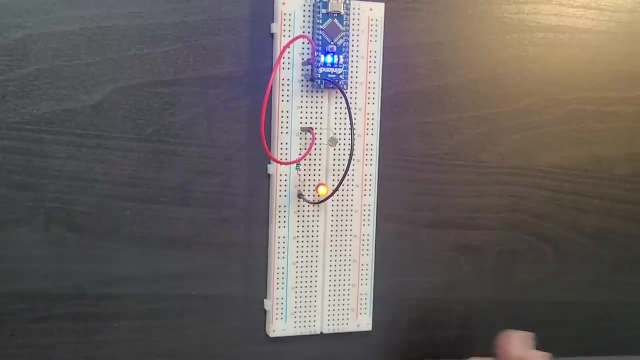 it's ready now, let me just turn it on. let's do that. turn it on right here. okay, everything seems to be working fine. let me just. everything seems to be working fine right now it does again. we're not going to be coding anything on the arduino, because we're just. 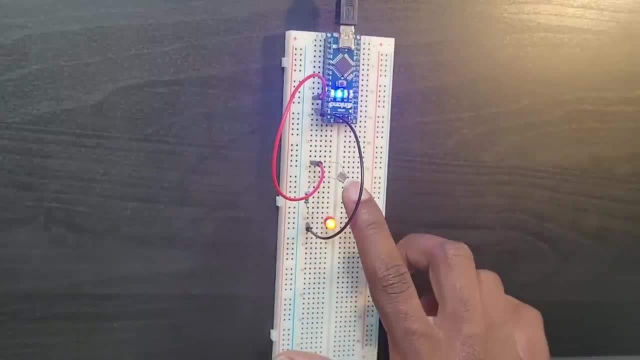 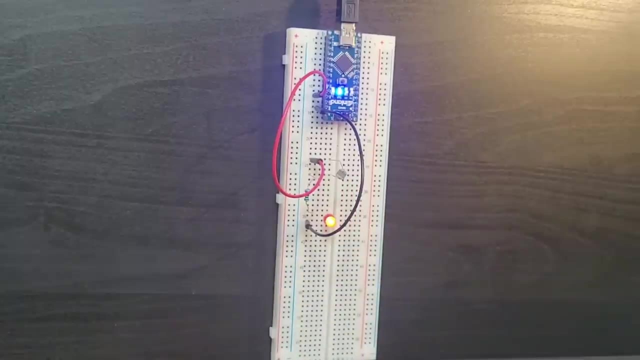 going to be using what? the 5 volt. so now i want to change what? the value of this, uh, this photo resistor, the value of the resistance again. right now i'm using what? two bright lights right here. i have one light right here on the left, i have one right to the right, so it's very bright right now. so clearly, the resistance value again. 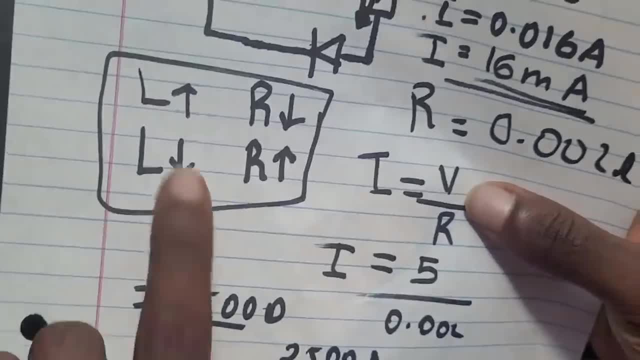 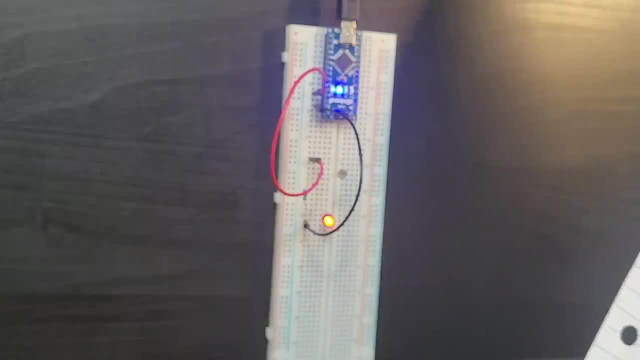 what happens? let me just bring my here: if the light goes up, the resistance value goes down. so in this case the resistance goes down, let's say theoretically, it goes down to very, very small number, let's even say to almost zero. okay, let's just say zero. so what basically happens here is: 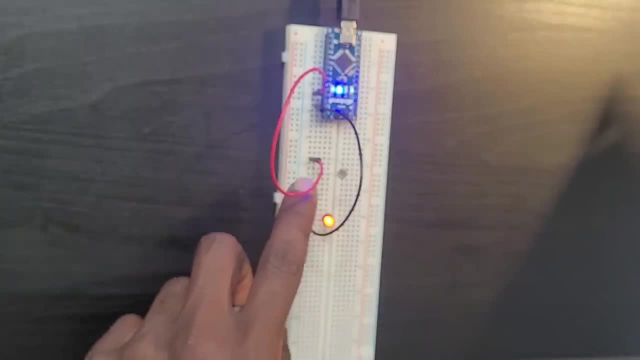 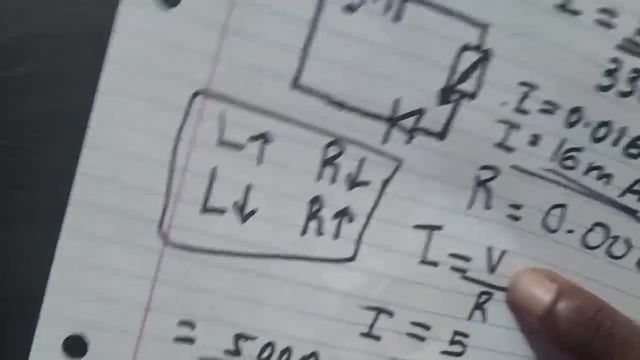 what we're going to have, our 220 ohm resistor. it's going to be obviously regulating what comes from the photo resistor, because in this case we're using what we're going to have: a very, very small number, almost close to zero. so we're going to have a very, very small number, almost close to zero. so 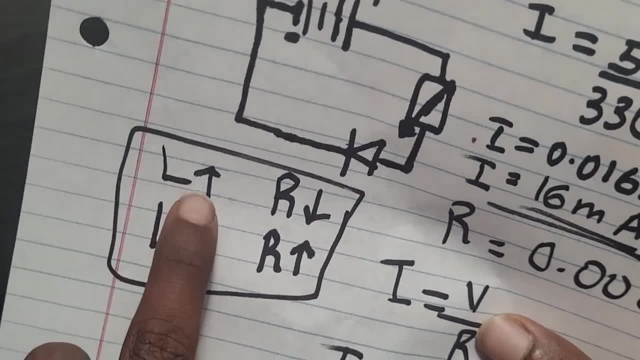 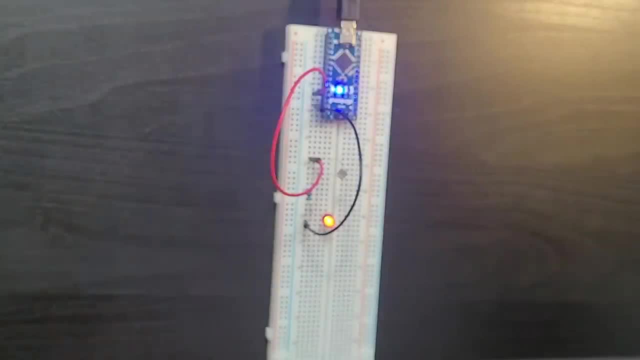 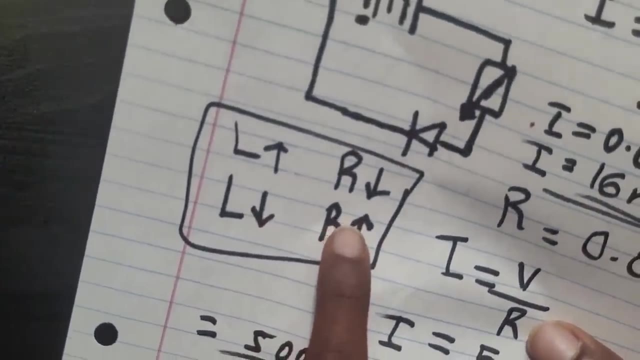 what? almost close to zero. okay, so light up. light is up right here, so the resistance value is down. that's why lots of current is flowing. so what? so our led is what our led is what our led is brighter. okay, so let me just try to decrease the light and see the resistance value come up. basically, 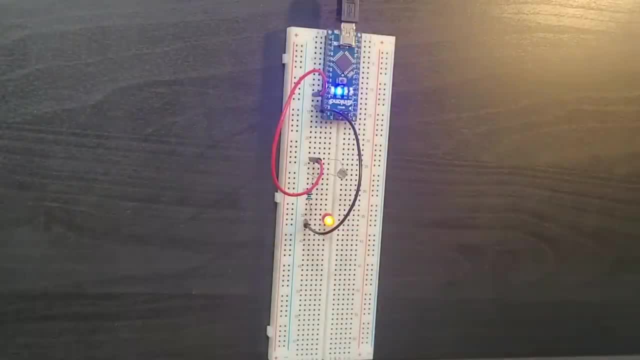 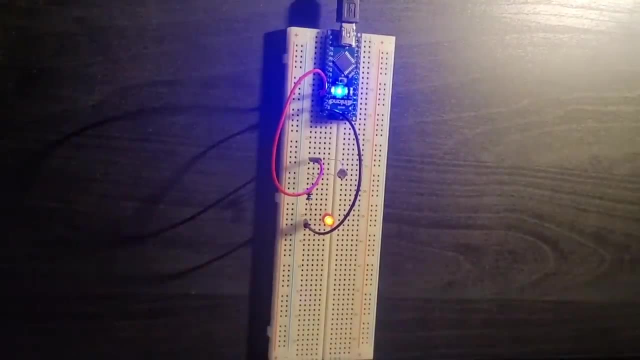 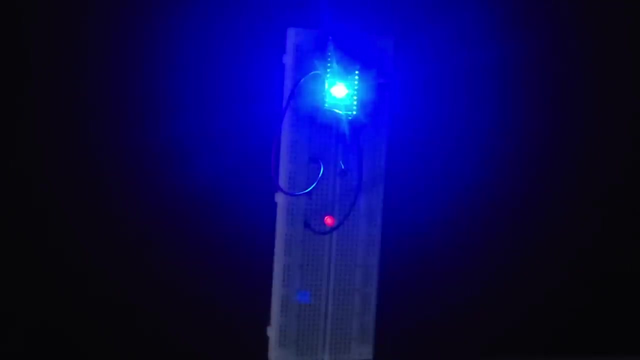 what? basically dimming our led? we'll just do that. so let me just go here, turned off one light, turned off both lights. it's getting dimmer. let me just go and even turn off the curtains. let me just fully turn them off. now we are in a very dark environment, except for the led that's lighting up right here. 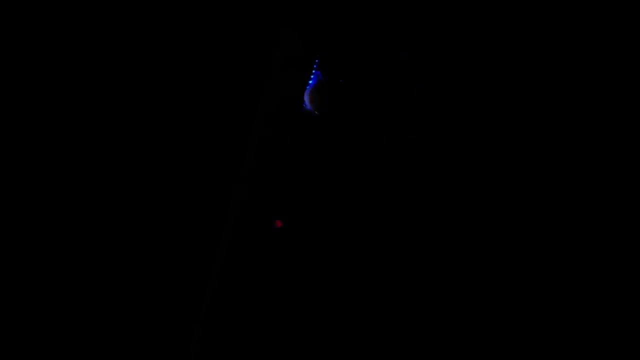 the arduino is built in led. let me just block it for now. okay, by my hand, you can see how dim it just got. you can barely see the red light right here. the red light right here. i just dimmed it out. okay, you can see that it's what. it's very, very dim. 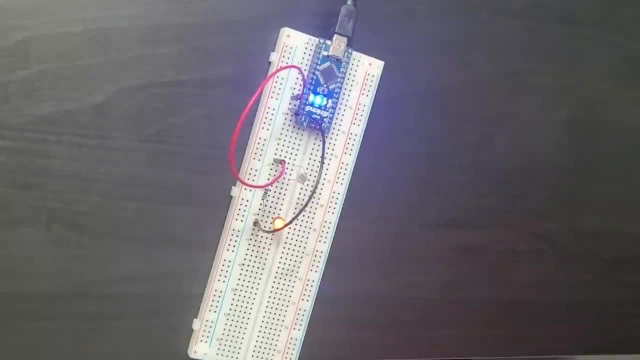 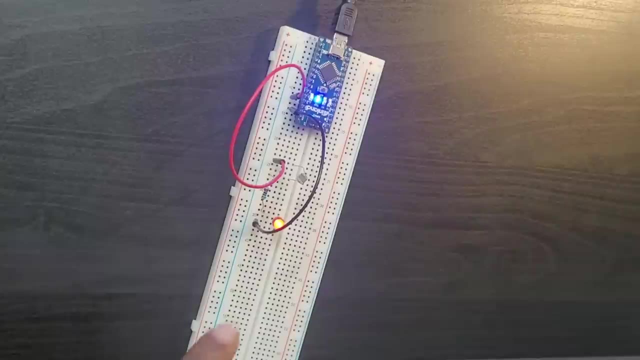 let me just turn on the light right now, both lights. all right, there we go. you can just see that what it was dim like a few seconds ago and now it's bright, okay. so this is one thing you need to keep in mind when working with what? with photo resistors, one thing we always keep in mind. 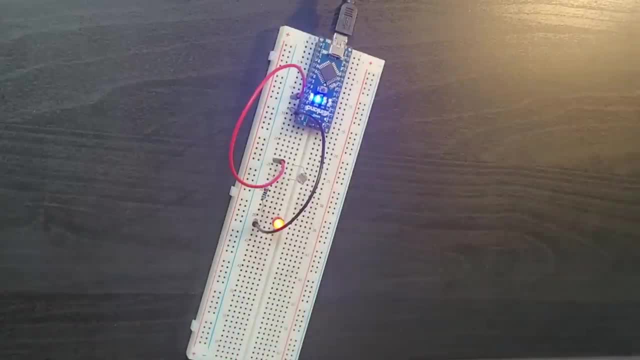 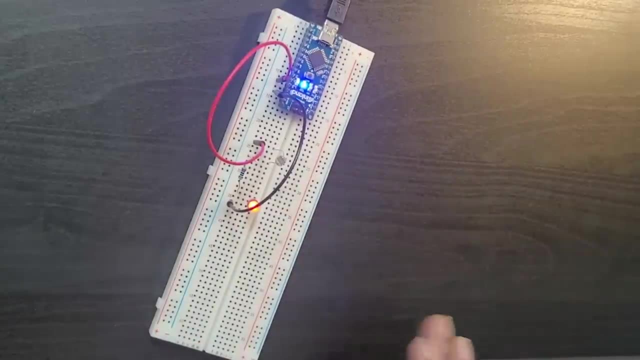 is what photo resistors are not always reliant. they're not always reliant. they're not always reliant on what they're not always reliant because? why? because again, there is this value: always changes by light. okay, so where do you think can we use these photo resistors? one of the applications: 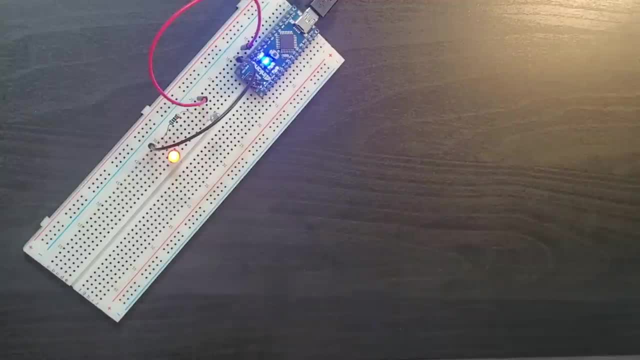 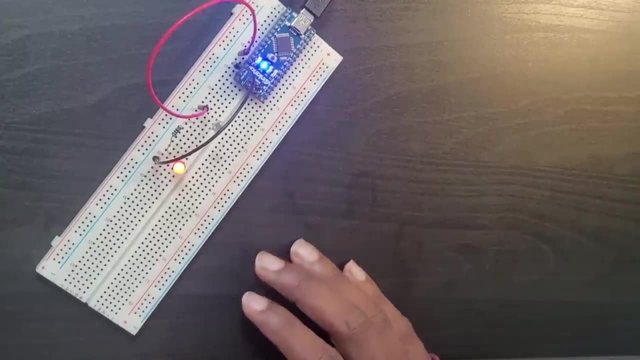 of foresters would be what, especially when we're using street lamps. basically, they're going to be what they're going to be: times where, again, street lights again will turn on and off automatically. again, no manual configuration, you, you don't need to turn it on or off. it's going to what it's going. 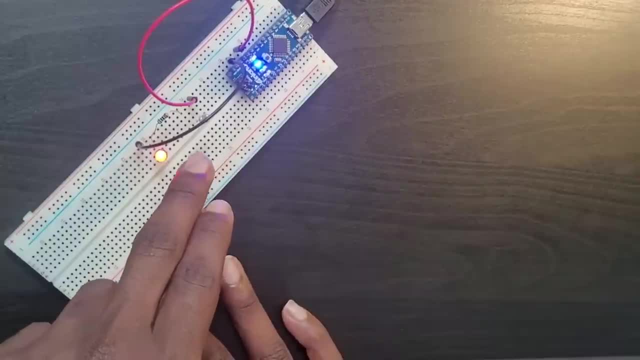 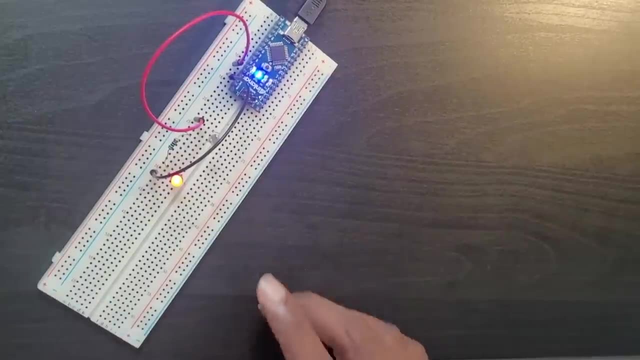 to detect the amount of light that is coming and out from the sun. and if it's very, very little, what's going to happen? again, the resistance value is going to be very high. it's going to record it and then then afterwards, it's going to what turn it on. it's going to basically what it's going to turn it on automatically. 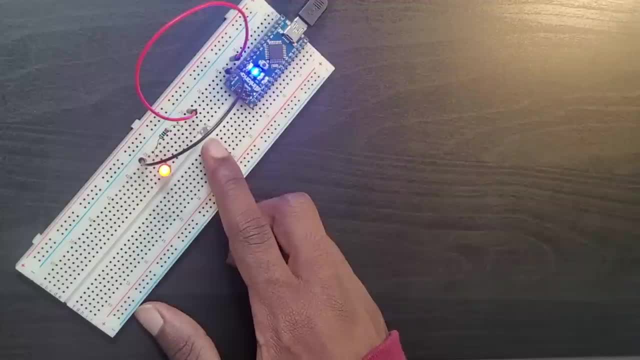 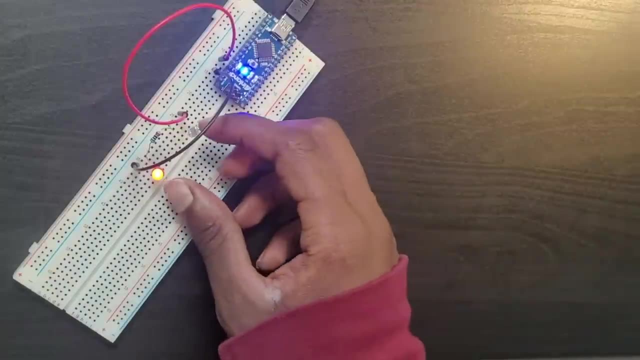 so we can use photo resistors for what? for soft, for self turning on and off lights? okay, so we're going to use them for what? for smart lights? okay, so we worked with the photo resistor right here. let's work with a bit on the thermo thermistors that we just 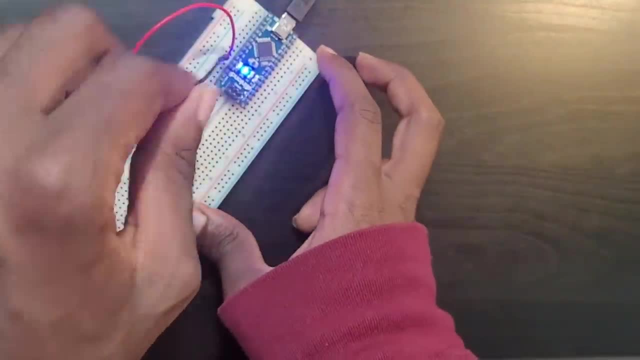 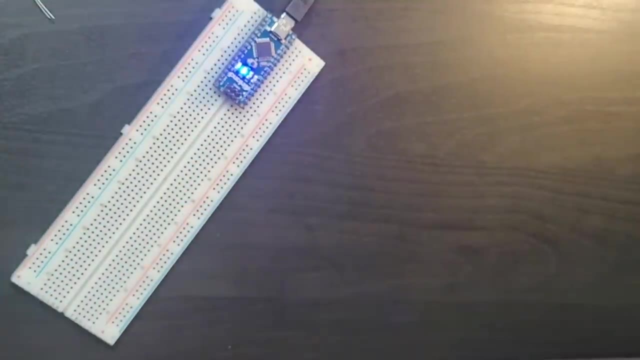 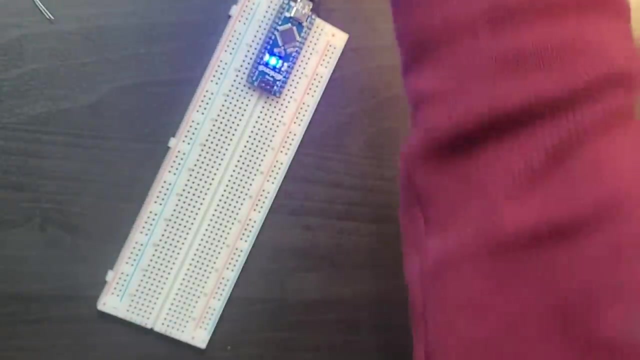 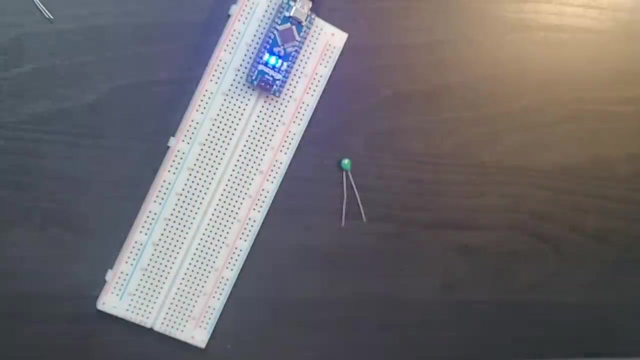 mentioned earlier. okay, let me just unplug all of this, take this off all of it. there you go, there we go. okay, just did that. and now let's spring my right here, my valuable thermistor, and let's try to do the same thing. so again, let's connect it- almost the same circuit. okay, let's try to do that. 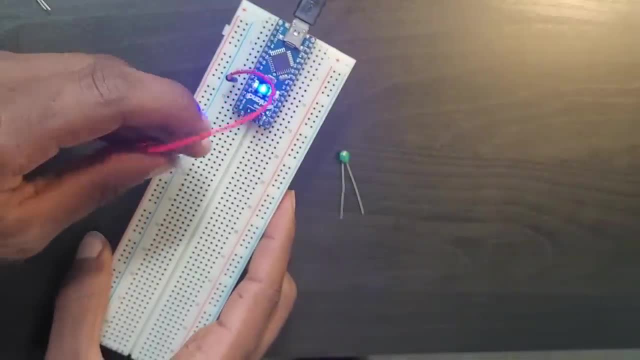 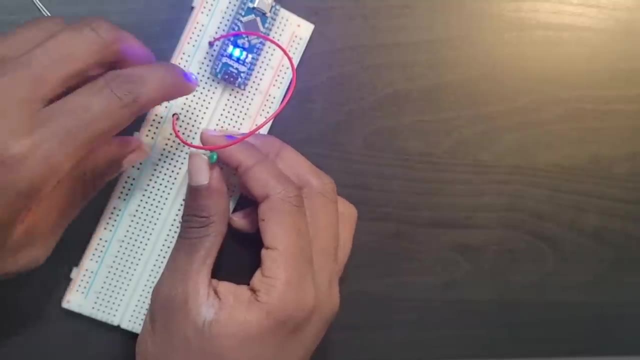 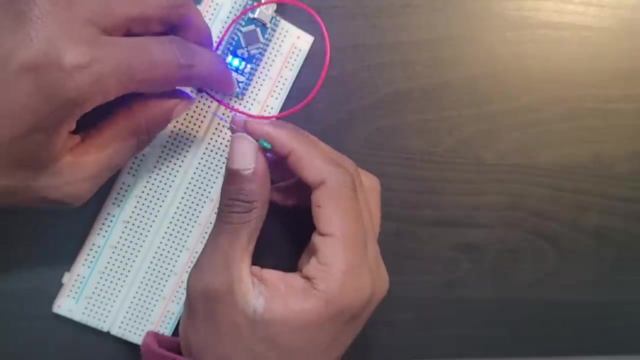 all right, i have my five volt right here, connected here. then i've got my thermistor again. i can put which leg i want to, because nobody's going to force me again, because it's not what, it's not important which leg you put it in. let me just go back here, get this straight. 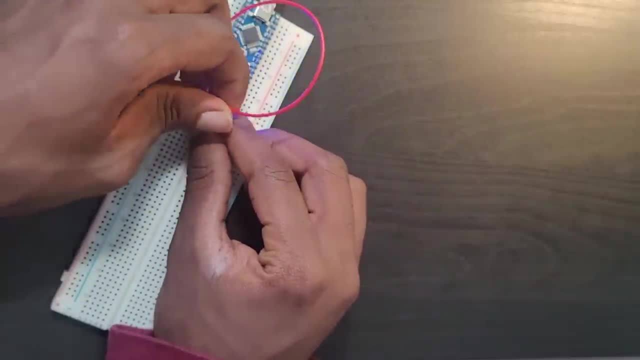 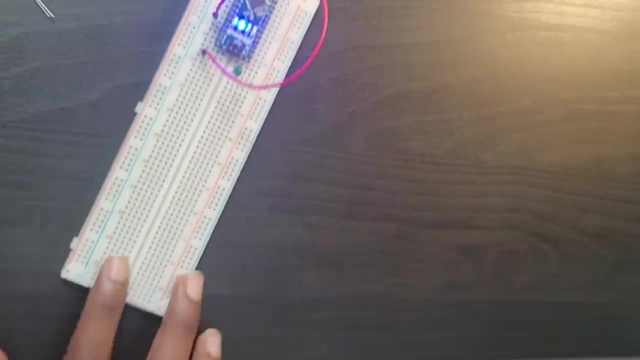 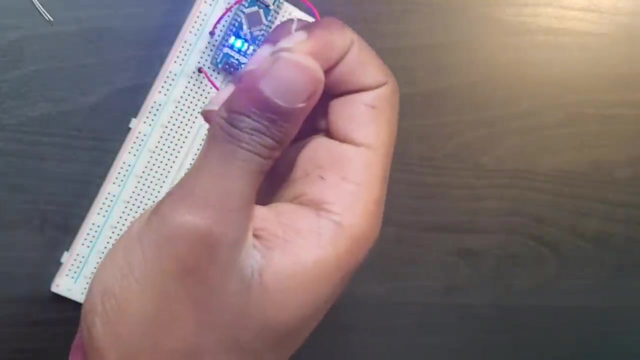 i actually put it here. just put it here, let me get it closer. i'm going to tell you why in a minute. i'm just going to put it closer to the Arduino, because i'm going to need this piece right here. okay, then, afterwards, what i want to do is use my normal again. my normal handy, again normal. 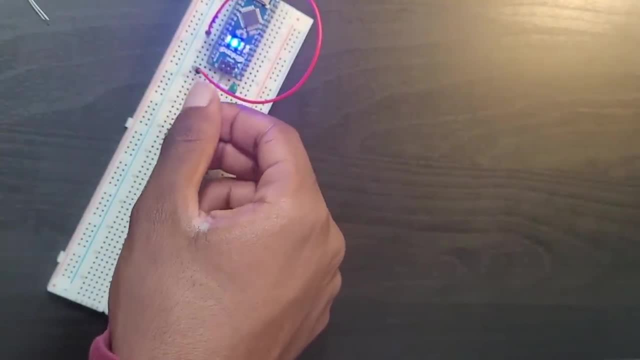 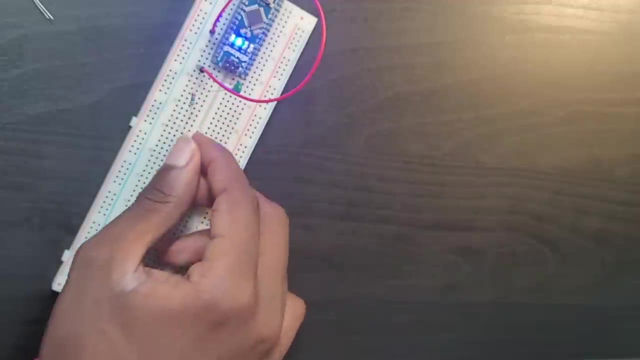 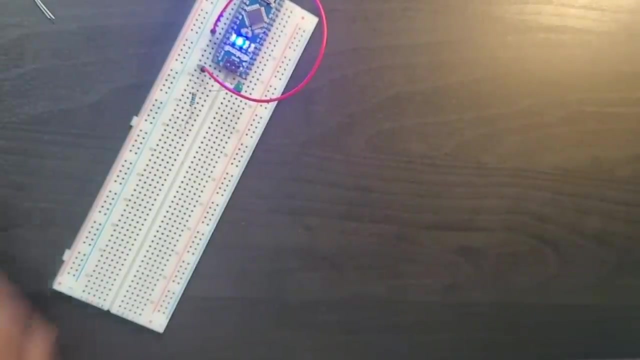 resistor. why is that so? because, again, the temperature value is going to decide if the resistance goes low or high. okay, so it's going to be very, very important for me to use what to use this so that i don't fry my led. okay, i did that. now what i'm going to do is what? 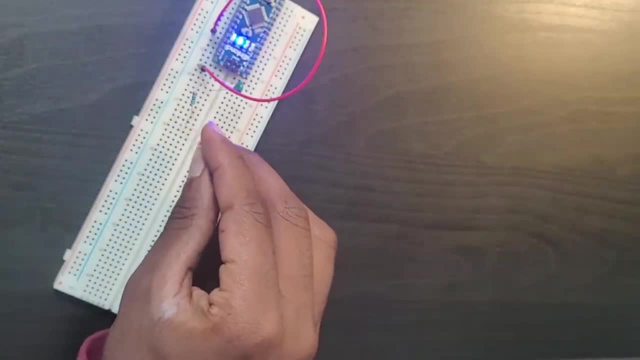 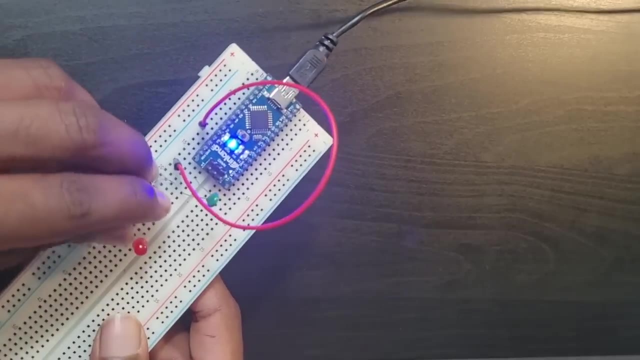 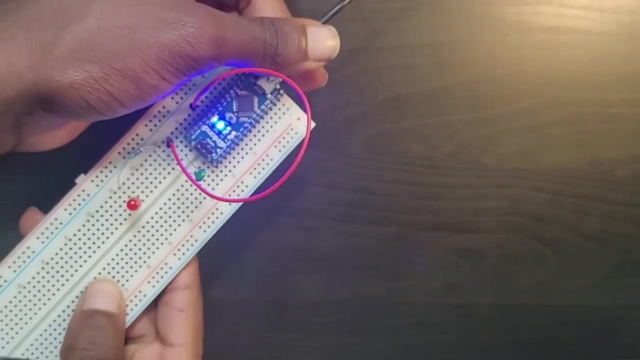 connect it to this edge right here. Let me just get this straight. The Arduino, the normal resistor, okay, it's acting. all right, there we go, It's connected. like this, I can just unplug my Arduino right here. There we go. Get it closer so you can have a better look. 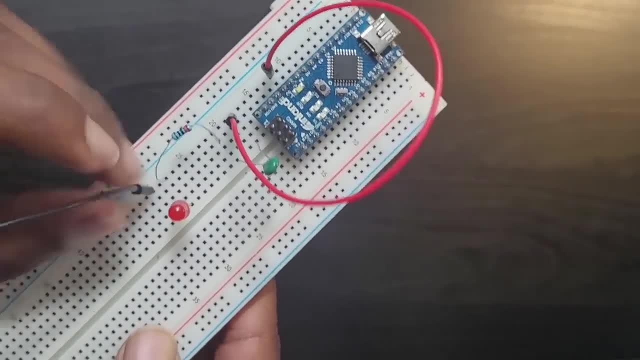 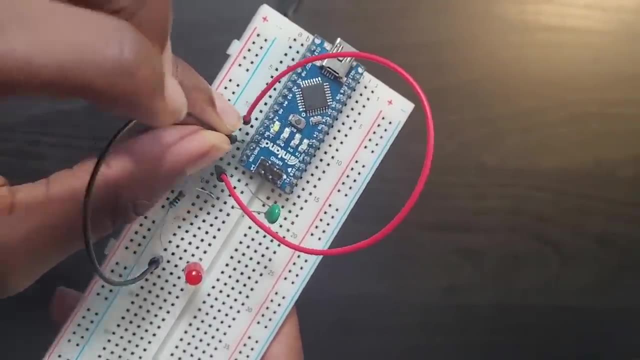 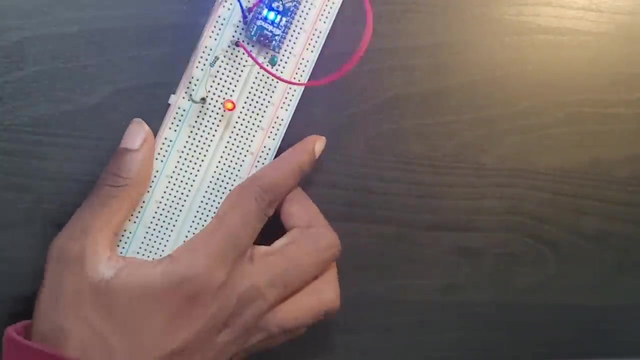 of it. Then I have my GND. There we go. Connect the GND to the GND pin. Let me just do that. All right. Now what do I need to do? Plug in my Arduino And you can see it's lighting. 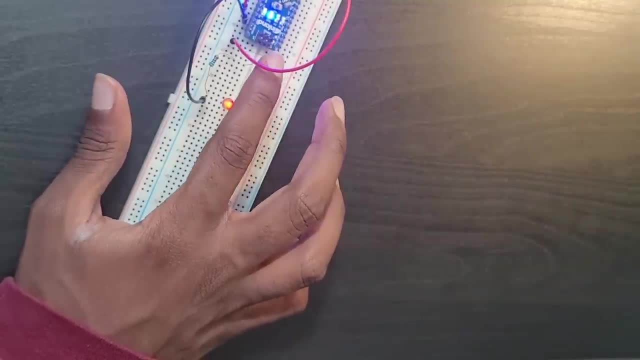 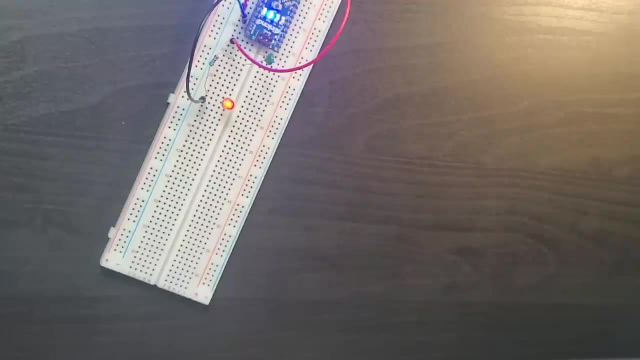 up a bit, Can you see it? So basically, temperature: here is what We cannot know yet. First thing now we have to do, Let me just bring another paper right here and try to explain what is going on. So let me try to explain what is going on right here. Let me get this out of the way for now to 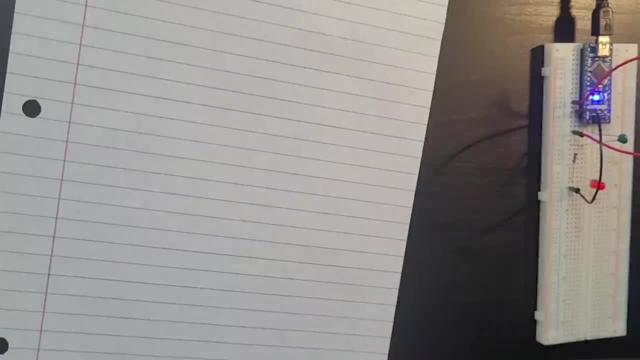 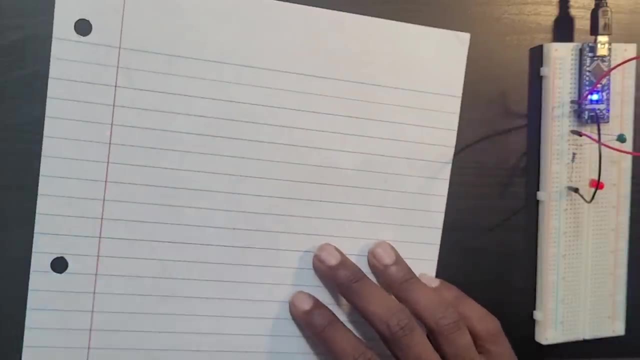 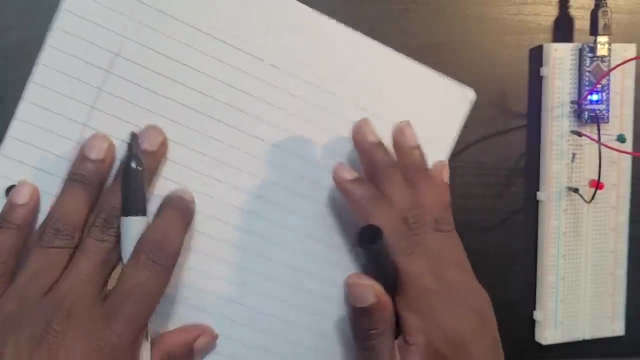 the edge of my photo resistor right here. All right, Let's bring my Sharpie right here and try to explain what's going on. So, when it comes to thermos resistors, as we said earlier, what did I say? I said that it's relevant to what is going to depend on the 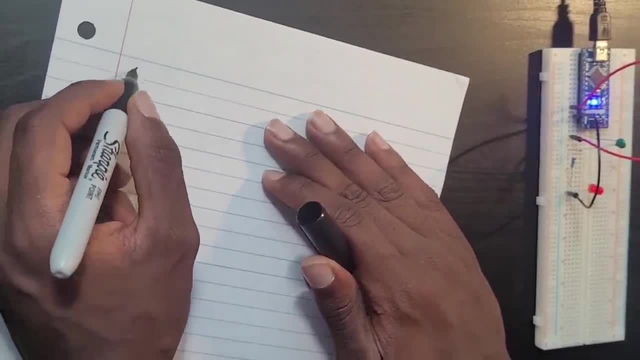 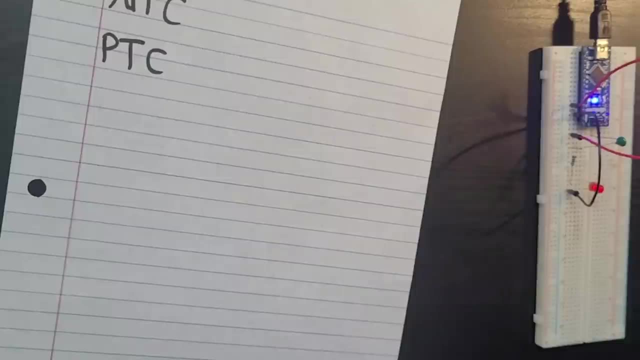 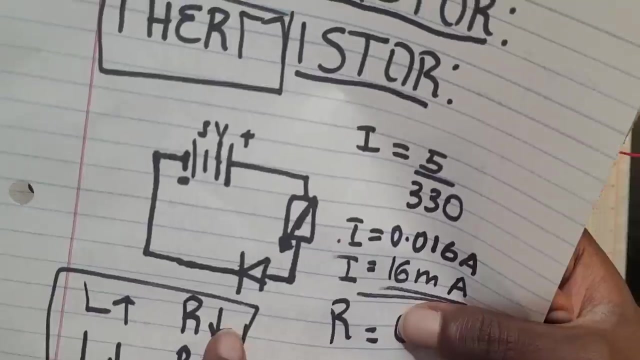 temperature. So there's something called NTC and PTC. So when it came to photo resistors, what did we say? We said directly: if the light is what? If the light goes up, the resistance value goes down. If the light goes down, the resistance value goes up of the photo resistor. 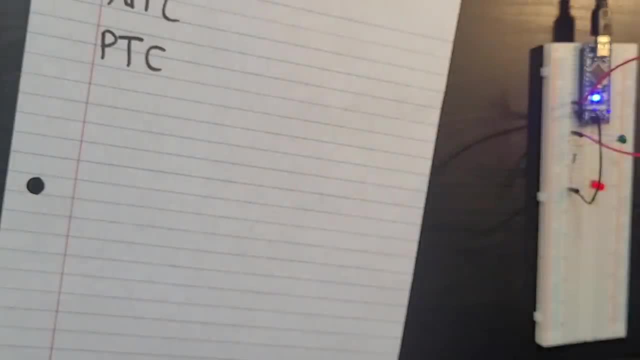 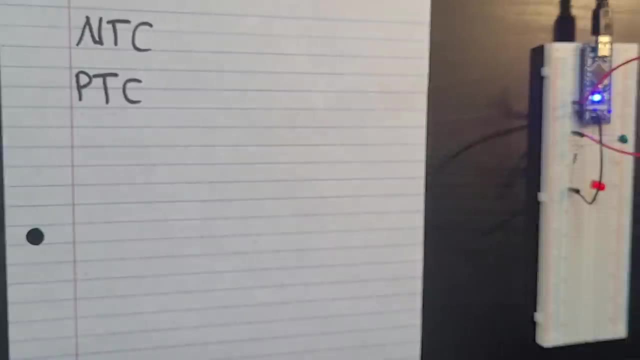 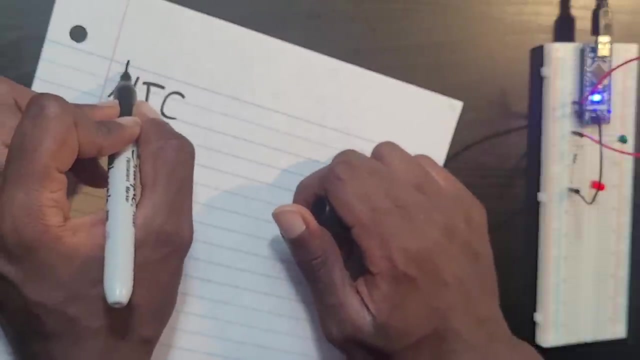 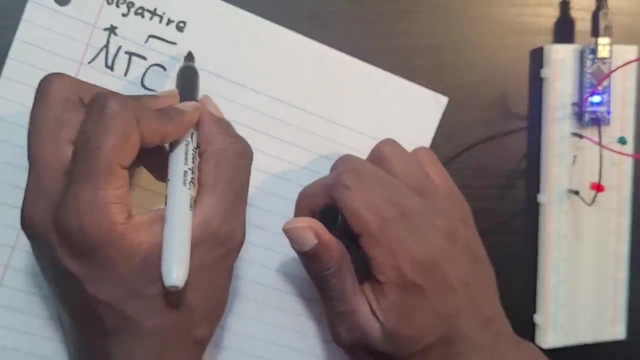 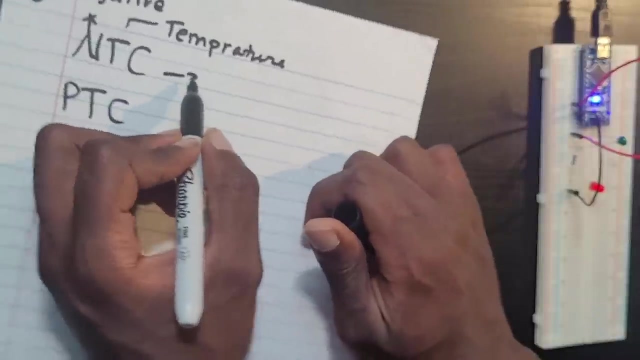 That's what we said for photo resistors. It was what It was. quite direct and straightforward. So when it comes to thermos resistors, there's something called NTCs and PTCs. N stands for negative, N stands for negative, T stands for temperature, C stands for what C stands. 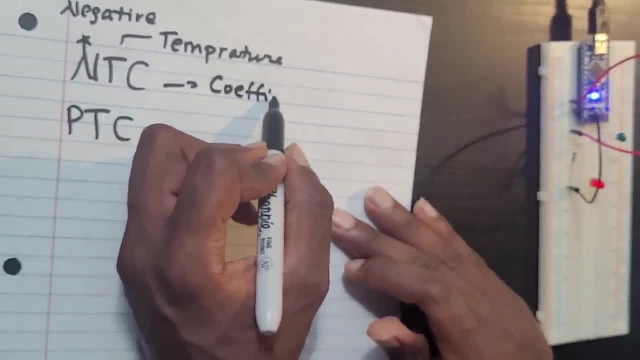 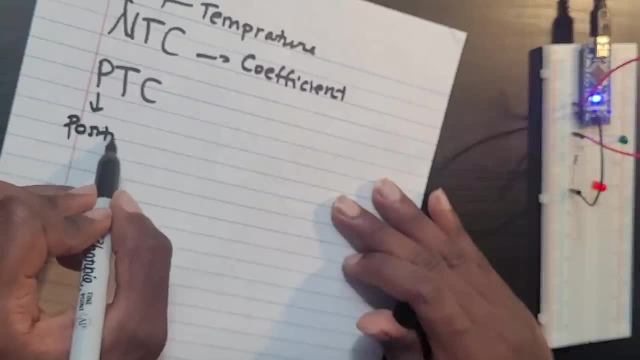 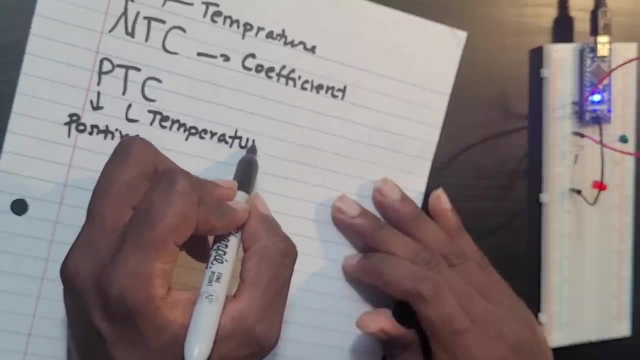 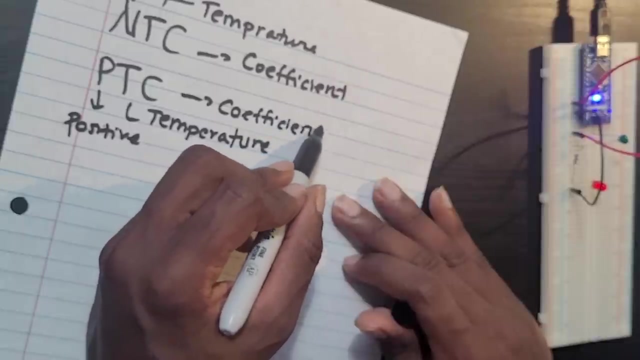 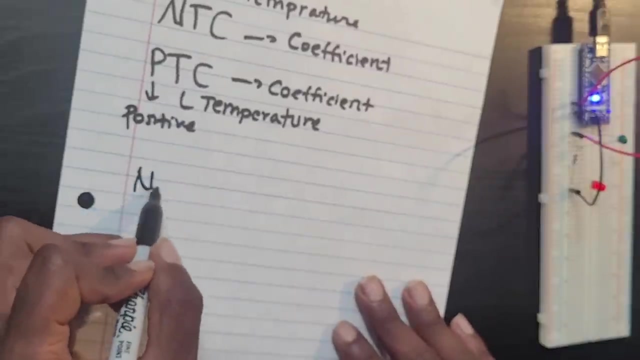 for control: coefficients: Okay, Okay, Okay, Okay, right here. coefficient: okay again. the p stands for positive- this makes sense right now. positive temperature: this stands for, again, coefficient, coefficient. let me just skip that. okay, so what does this mean? so, when it comes to ntcs, right, one thing to keep in mind is when: 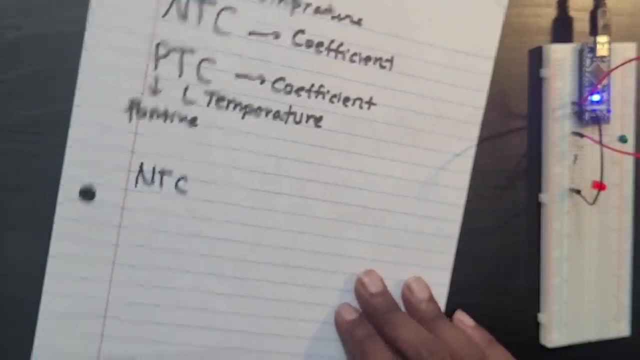 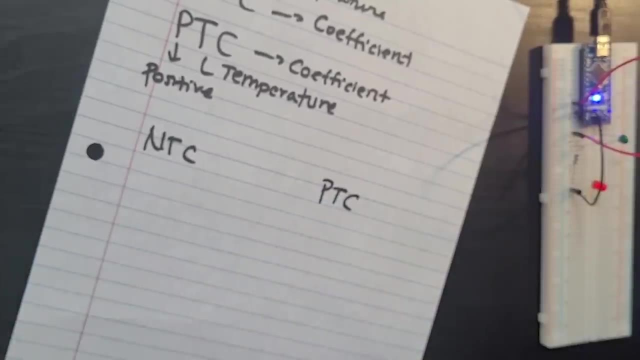 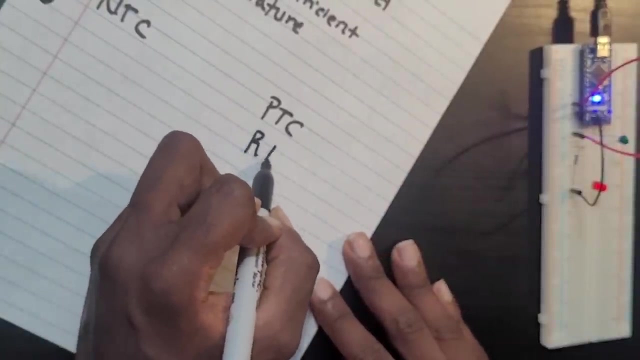 it comes to ntcs, is that okay? when it comes to entities and ptcs, is what? they're both affected by temperature, okay, but the difference here is that when it comes to ptcs, what happens is resistance value. it increases. by what? by increasing temperature. okay, so the resistance. value increases. by what? by the amount of the temperature. right here, when it comes to ptc, to the ntcs, what's? uh? it is what. it's opposite. so the resistance value: what increases per decreasing temperature. so as soon as temperature starts to decrease, the resistance value, what starts to what increase? 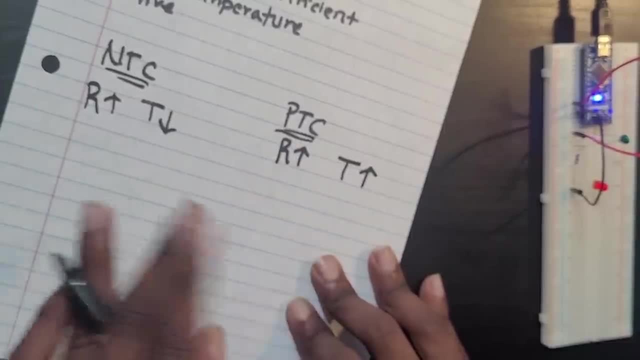 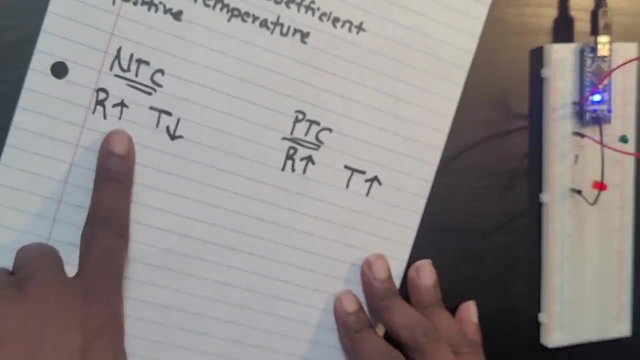 again, this is what, due to the material they're made from, they're made from different materials. so, again, in this case, the resistance goes up while temperature goes up. in this case, the resistance goes up while temperature goes down. again, we can put this. again, we can put the inverse of this. so, 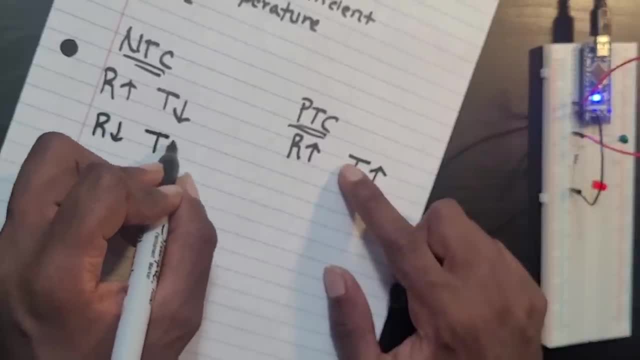 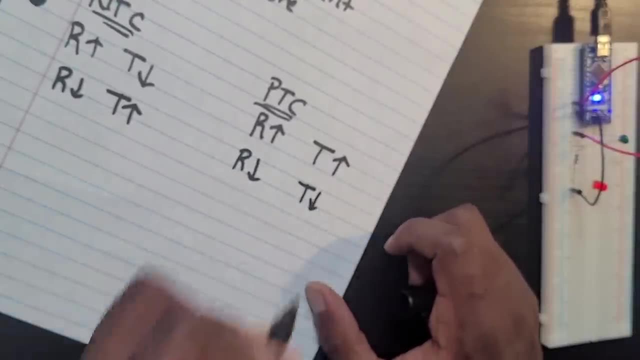 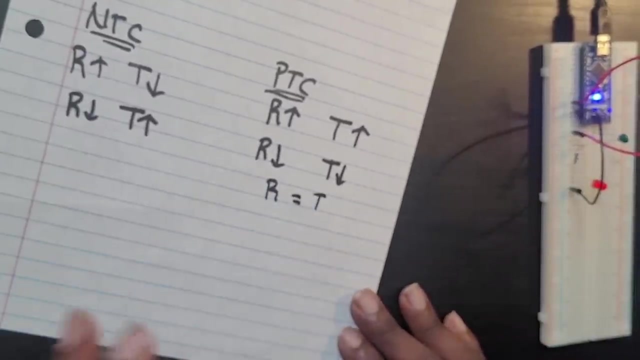 the resistance goes, what down when the temperature goes up. we can say, for this one too, there is this: what goes down when the temperature, what when the temperature goes down? okay, so in this case, what the resistance and temperature have, what somewhat of a what? they're directly proportional. 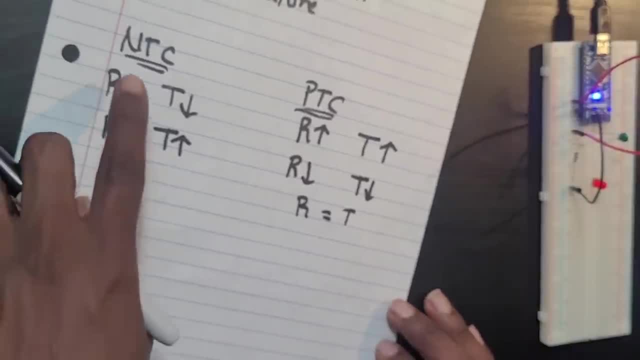 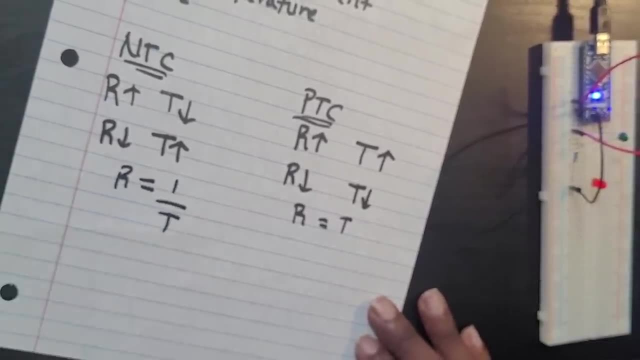 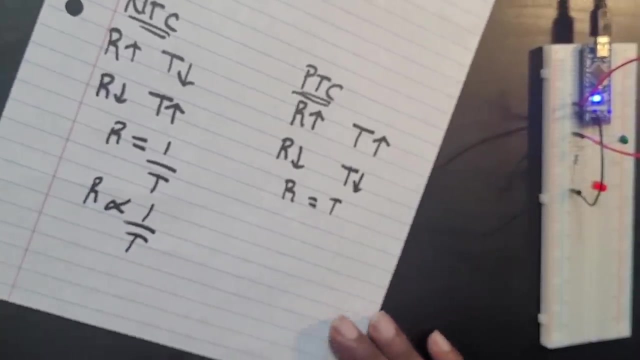 basically, they have a what a straightforward relationship, while in ntcs, what do they do? they have an opposite. they have an opposite, what they have, an opposite, an opposite relationship there's. we can say: r is what? indirectly proportional to what? to one over t. we can say: 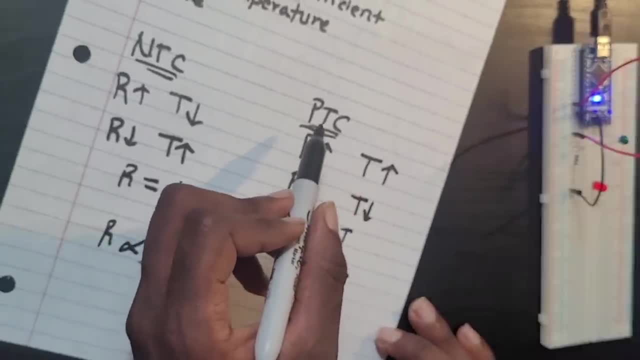 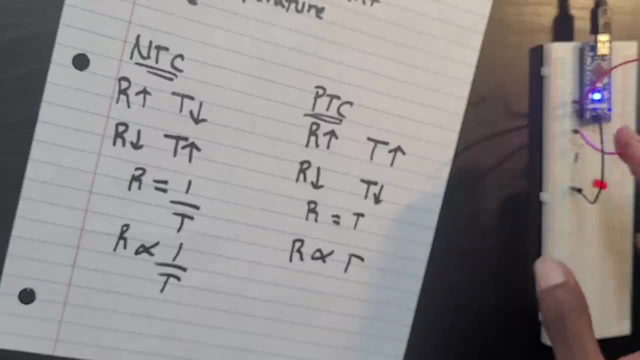 r is directly proportional to t, or what, or positive what temperature coefficients. so so that it depends on what, it depends on the, on the thermistor we have here. it can be ntc or it can be ptc. okay, so while keeping that in mind, right, one thing i wanted to do here was: you know what i want to check if the 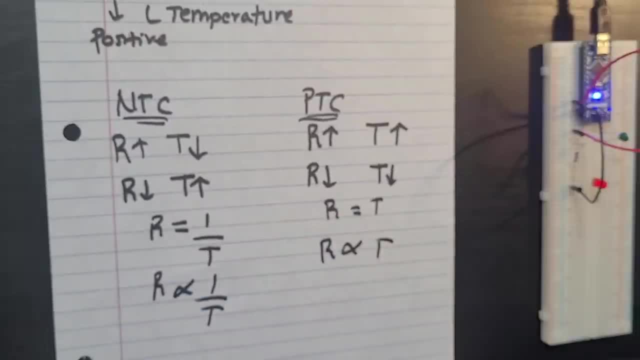 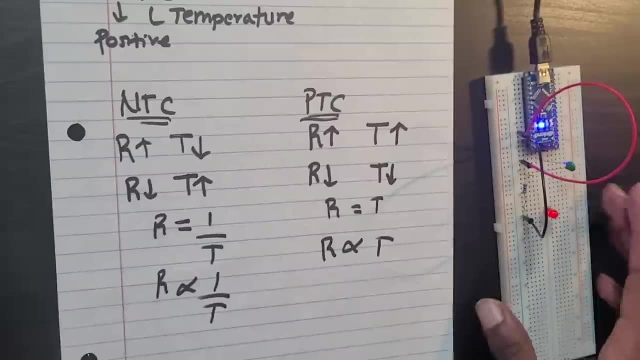 temperature goes high or low, but the problem being here is i have to use something that has big source of heat, and i don't want to get this what close to my arduino, because it can want, it can ruin my arduino. i don't want that to happen. that's why. 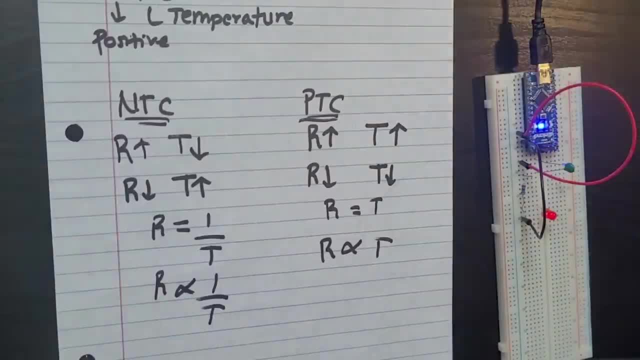 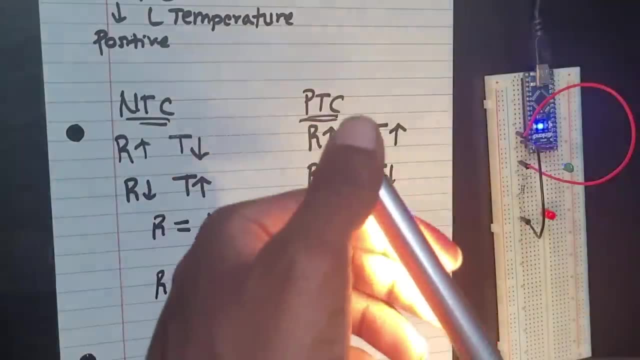 i'm just going to be using the light, so i'm going to be using light. i'm going to be using a normal lamp here, and this lamp heats up, especially in the back. let's heat it up right now. oh, it's a lot, it holds a lot of heat here. 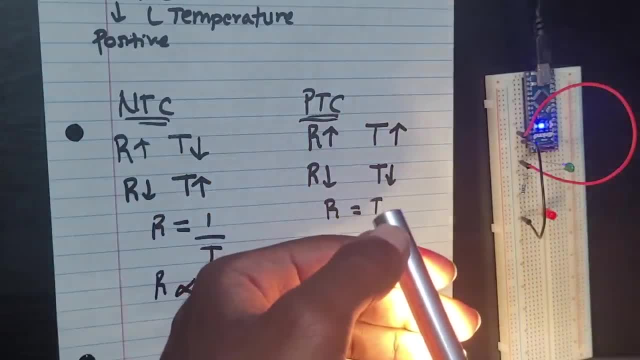 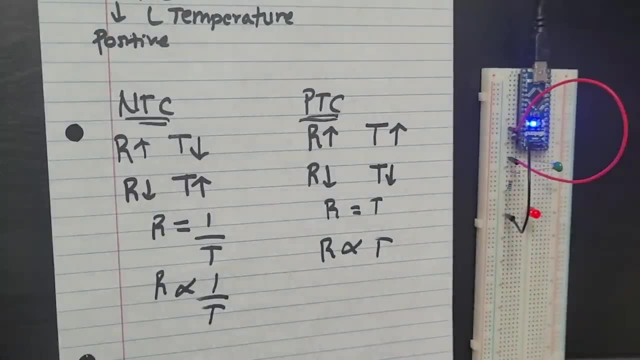 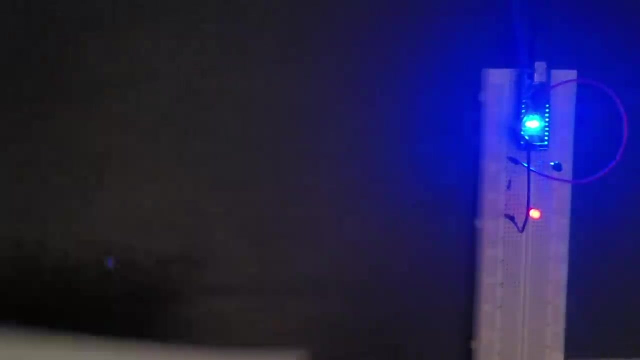 there's a lot of feet here. there's a lot of feet here and i want to do is just get it close here so we can see if the- uh, if this one, changes or not, if the led changes or not. okay, let me just turn off my light. this light, i'm gonna need one light only. let me just remove this for now, because 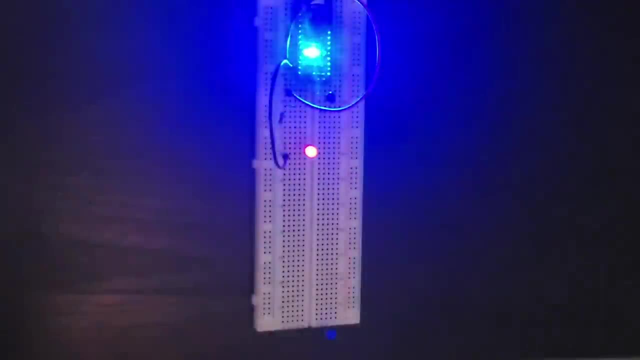 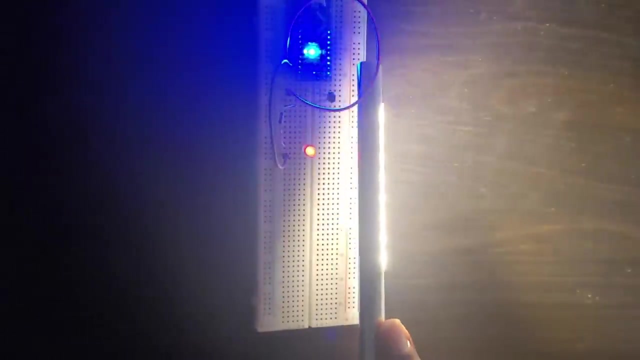 we don't need it now. i'm just trying to get with the light on. what i want to do is again get this so close to the what, to the light, and then i'm going to turn off my light and i'm going to turn on the thermistor so that maybe we can see a difference: the what in the led. 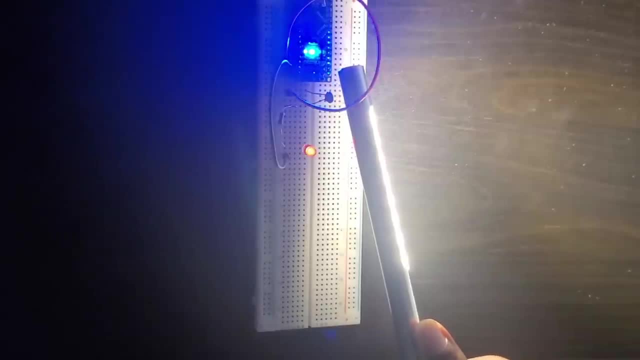 do you see a difference? i can't, let me just do that. i keep trying to, but i don't see any difference, barely even see any difference. there might be a difference, but it's going to be very little that we cannot see it in our eyes, both of us um. 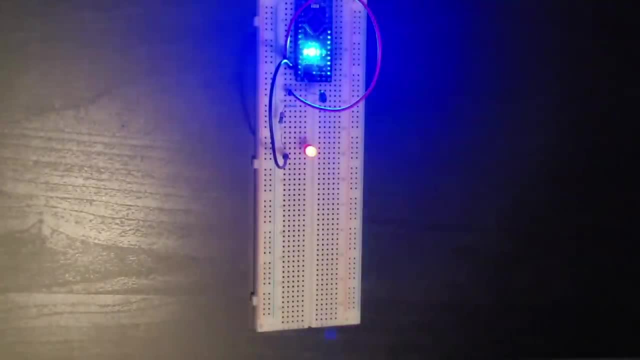 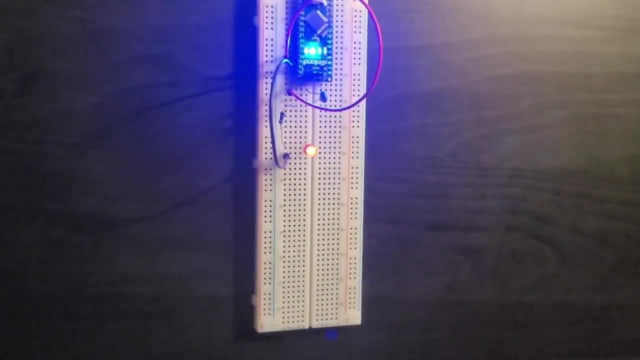 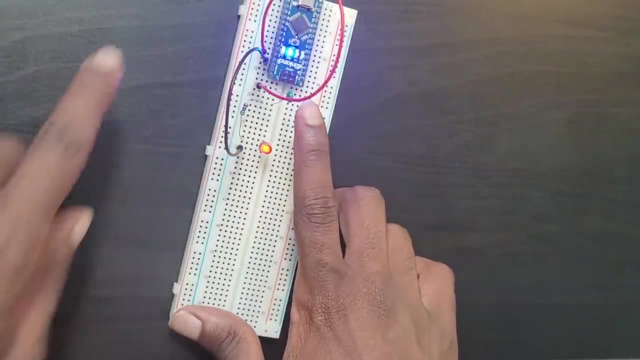 so one thing i want you to keep in mind right now is: okay, i want you to keep: all right, let me turn on my lights right now. for now, let's turn this on right here. and this one on one thing i want you to keep in mind is this: thermistor does not change very easily. why is that so? this one. 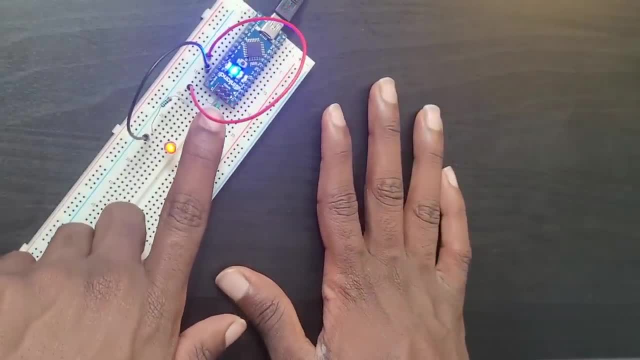 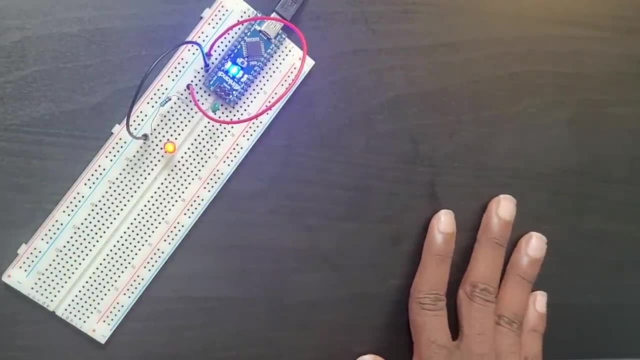 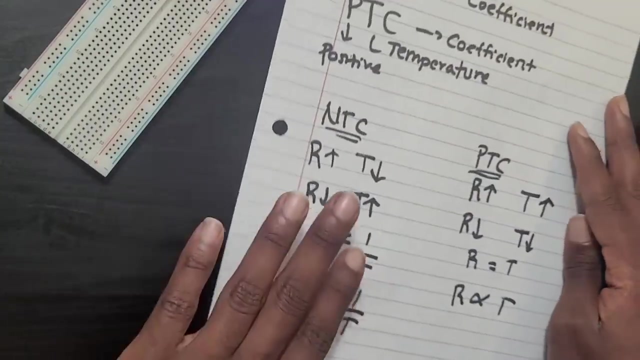 specifically again. check your label specifically. this one has 10 000 arms, so what has 10 000 ops? the is big, so it's going to change. for what? for bigger temperature, okay. so i just want you to keep this in mind again. one thing i want you to keep in mind- it's not about the i want you to keep in mind is: 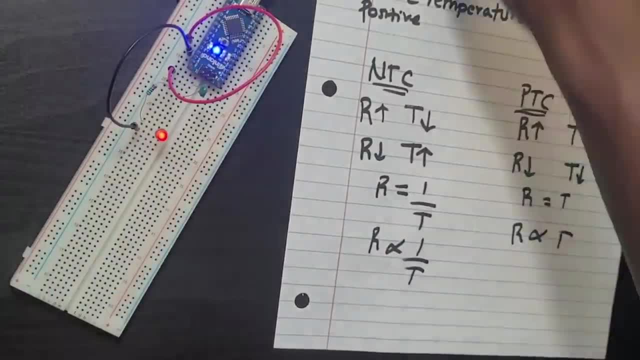 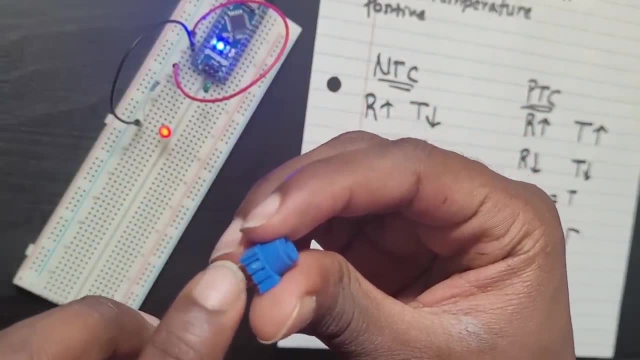 all right, right here. this has 10 000 ohm resistor, just like how the potentiometer has a total combined of 10 000 ohms. again it has 2 000 ohms, 10 000 ohms of resistance. this one has a 10 000 ohm. 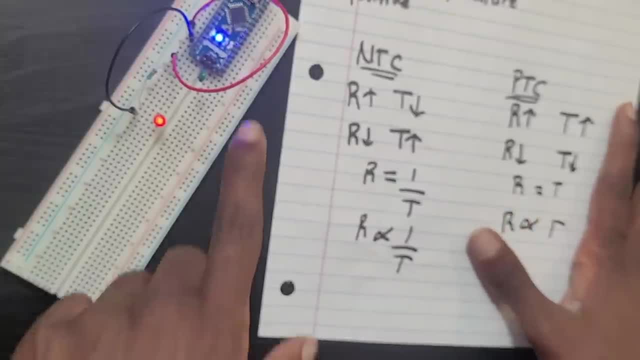 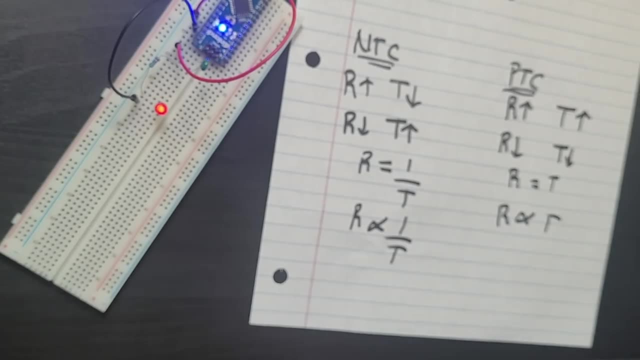 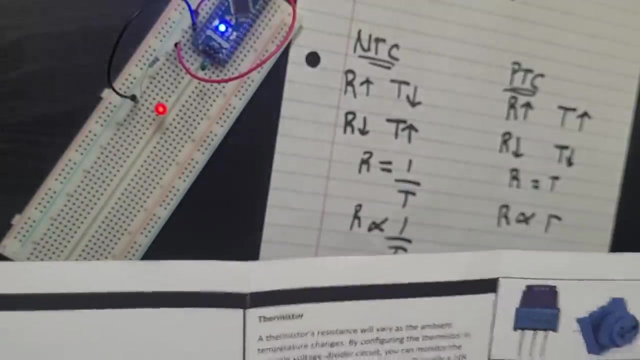 of resistance too. again, i checked the what, i checked the label, the label. and then i checked the. has it written out? because it just says 10 000 next to it. okay, on the label, okay on the paper that i just had, my what my arduino kit just basically sees it here: 10 000 ohm. it's going. 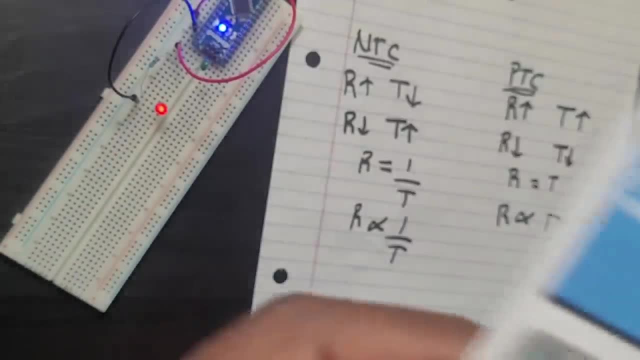 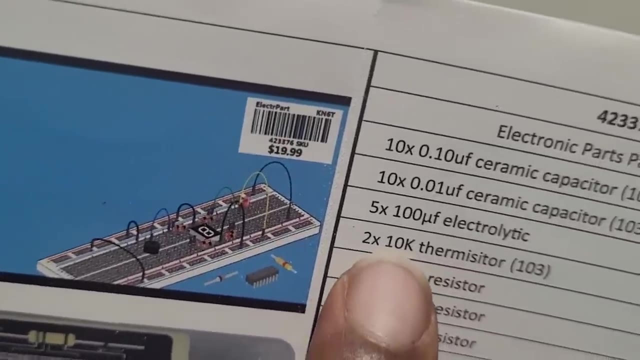 to go to components right here and all i need to do is go to components and be like, oh, there we go, they have a thermistor right here. it has what 10 000 ohm. i have two pieces of what 10 000 ohm. 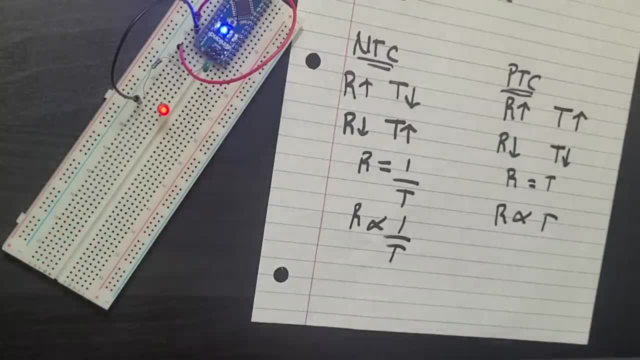 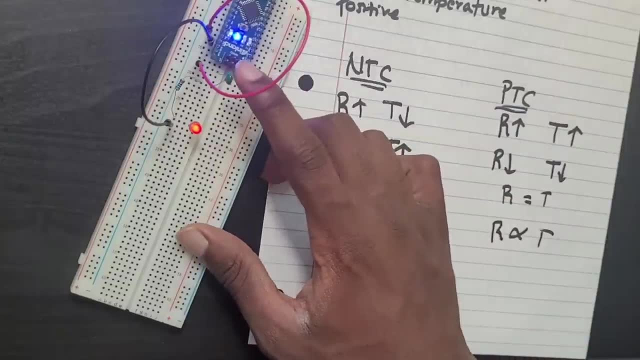 thermistors. okay, so this is what: 10 000 ohms, very, very big number. so what? so we cannot change, though we have to change the temperature very, very, by very big numbers. i'm talking by very big numbers for us to see a change in what. 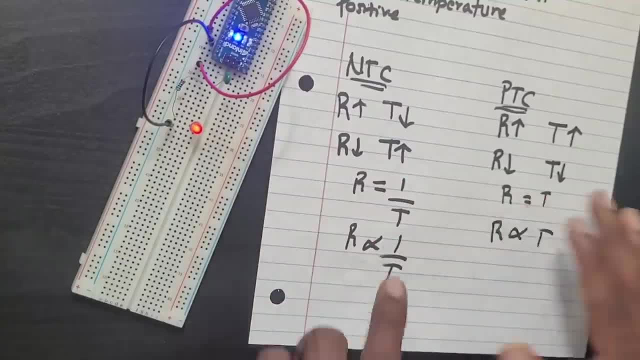 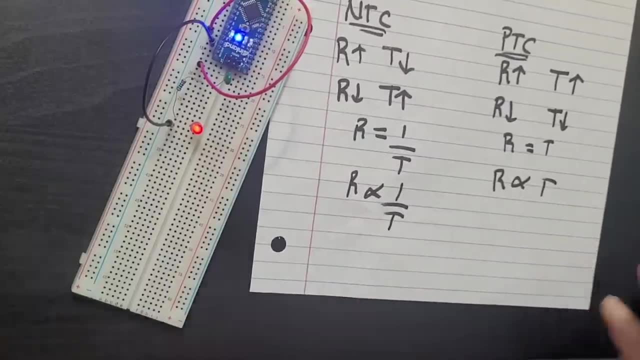 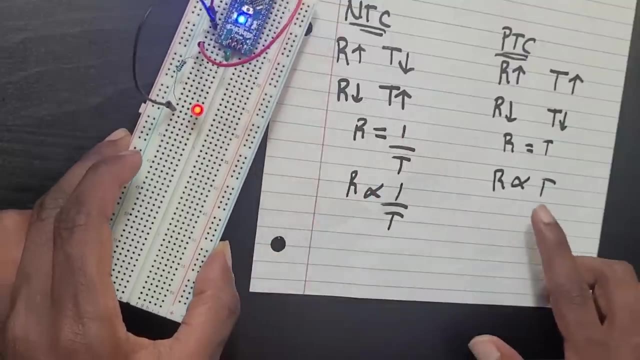 in the resistance. because, again, why? because i said again, either they're very, they're related directly or they're related to what indirectly? okay, so one thing to always keep in mind is what? oh, one thing to always keep in mind is what the resistance is: either directly related. 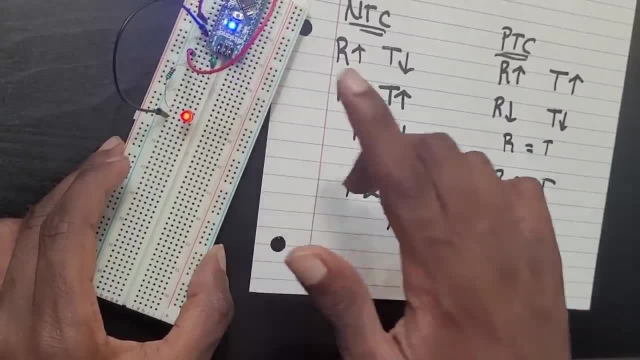 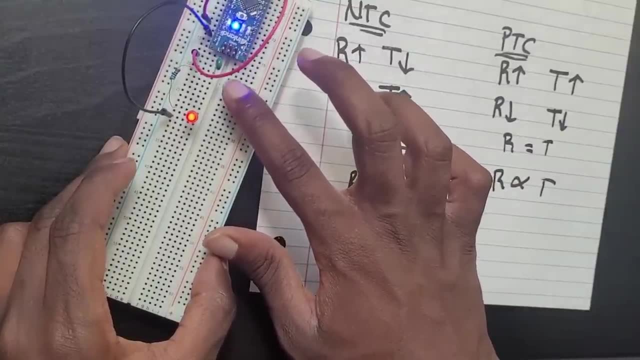 directly related to temperature. so right here, 10 000 ohms is a very, very big number. so we're going to have to change it by a very, very big number, by very, very big temperature, for us to see a difference in what in the resistance. basically, we're going to have more current, so we can see. 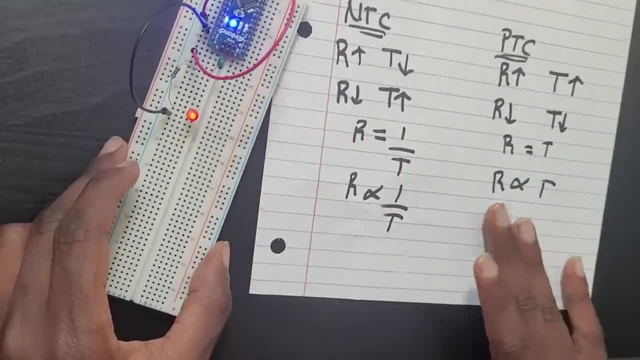 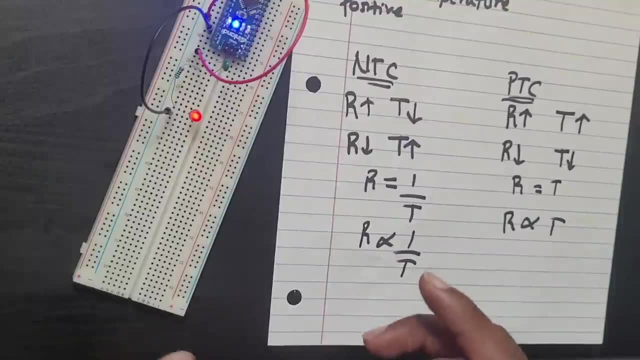 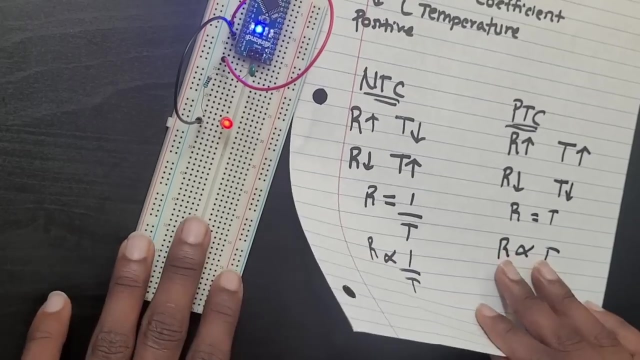 the light here so we can see the led here. just keep that in mind. that's why i'm going to need to maybe use- uh, if i can match- and sticks or something that is so hot so that again this can change in value. but i just don't suggest that you guys do that. if you want to do it, i highly. 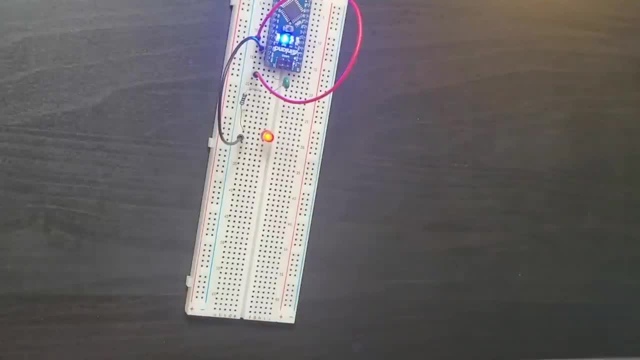 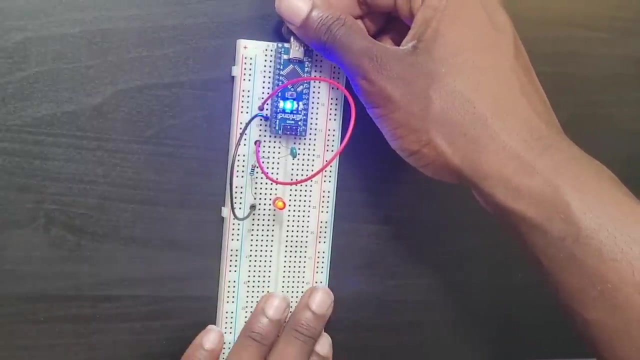 suggest that you guys use of a digital again, those digital arduinos or simulators again, because you don't want to get hot stuff near to your again electricity. this is not what recommended specifically, especially for kids. so, uh, don't do that as far as you can. don't do that, all right. but 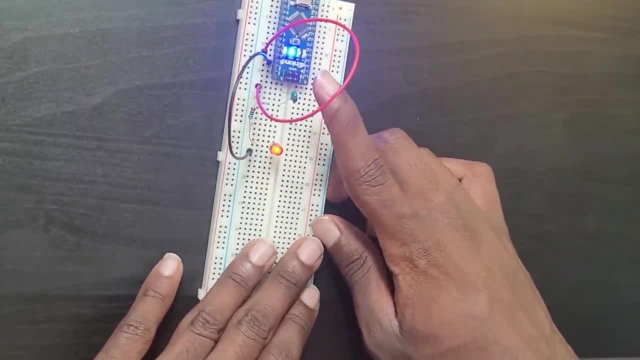 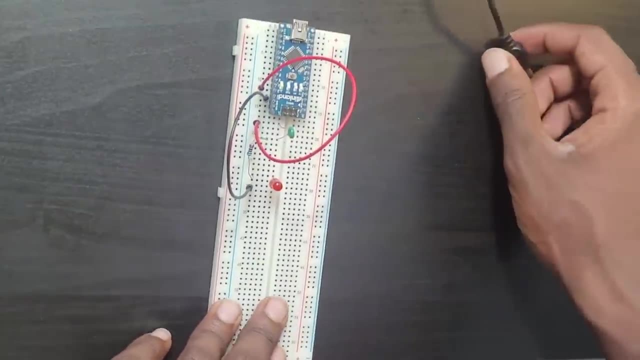 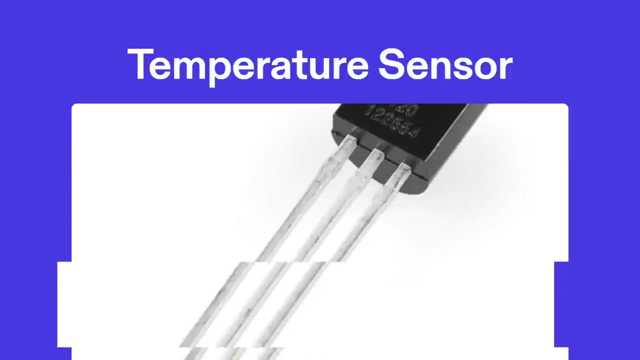 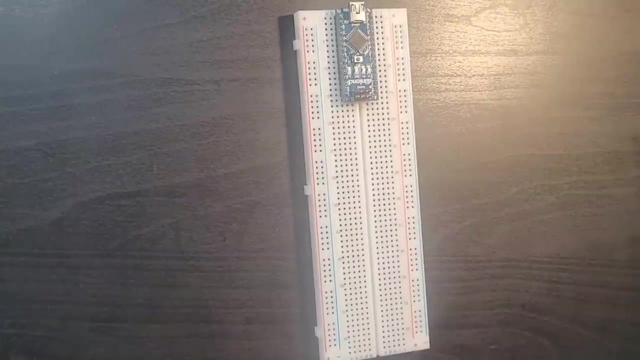 one thing you need to keep in mind is what thermistors always change in, what they always change according to what temperature. just keep that in mind. all right, this was a bit of a long one, so um see you in the next section, actually. so um see you there, all right. so now let's discuss about, uh, temperature sensors. so 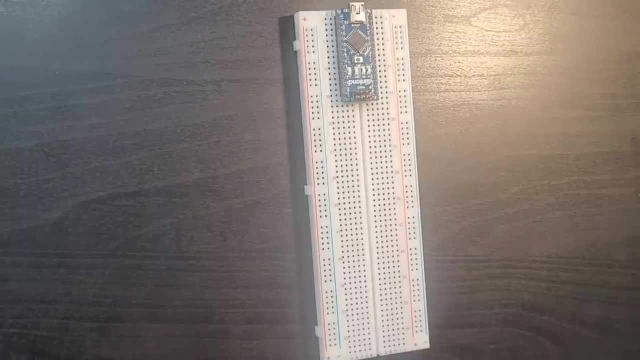 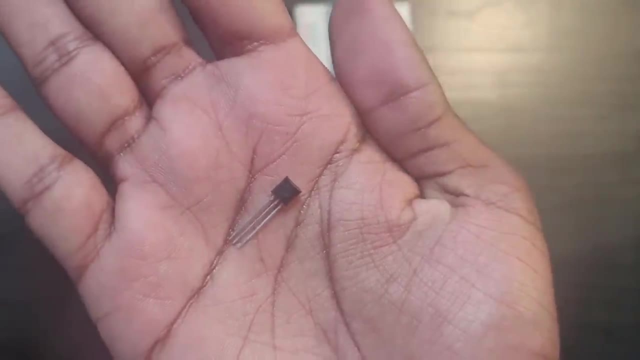 so far, we've not discussed about any sort of sensors, and this right, of course. so this is going to be our first sensor that we're actually going to talk about, so let me just bring this closer, so you're going to get see it. so this is a temperature. 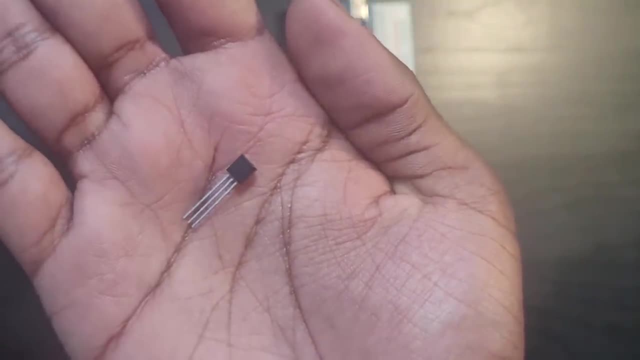 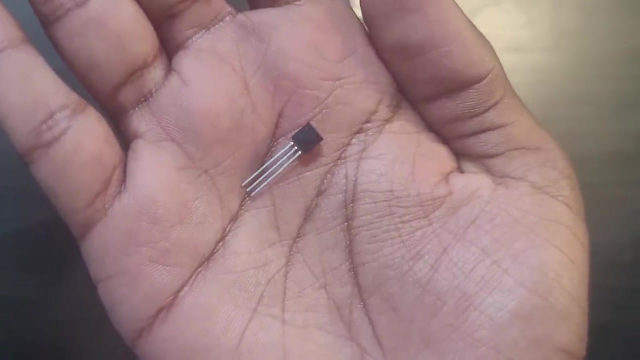 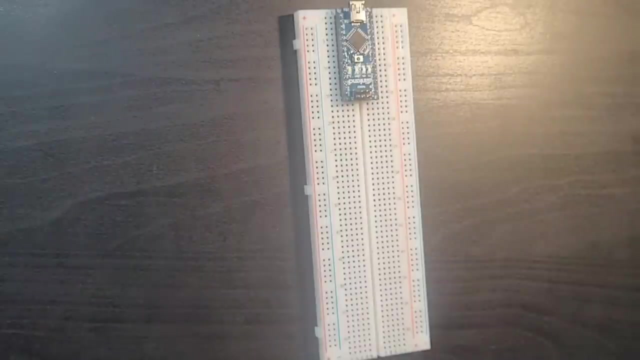 sensor, specifically called the lm35, and you might have a different type of sensor depending on, again, your arduino kit, the arduino kit that you have, but first, though, we're going to see how you're going to know what type of sensor you have, so, obviously, the first and the best method to know. 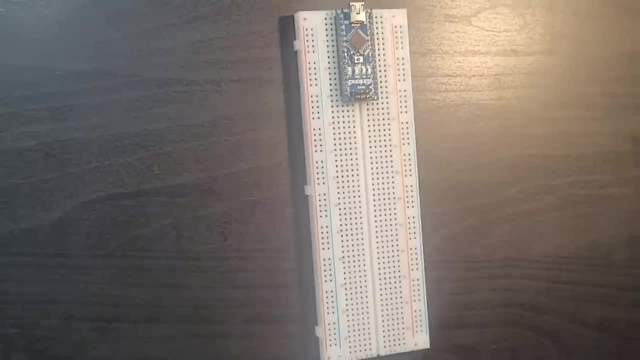 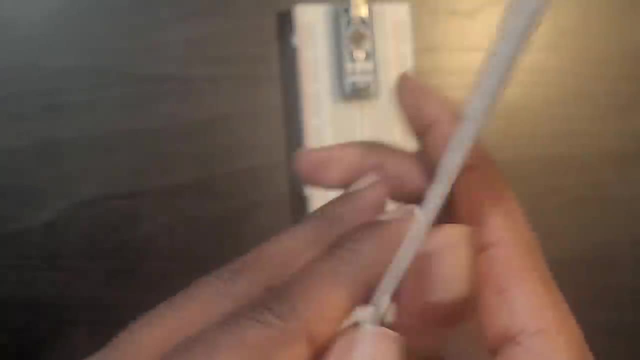 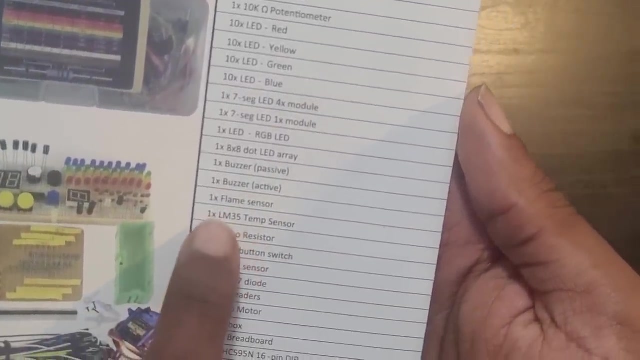 is always again reading the manual, okay, so i'm just going to bring my manual right here, a manual that i got my kit form kip from, and what i'm going to do is search for the components right here. and when you read right here, it says one, one piece of what: lm35 temperature sensor. okay, 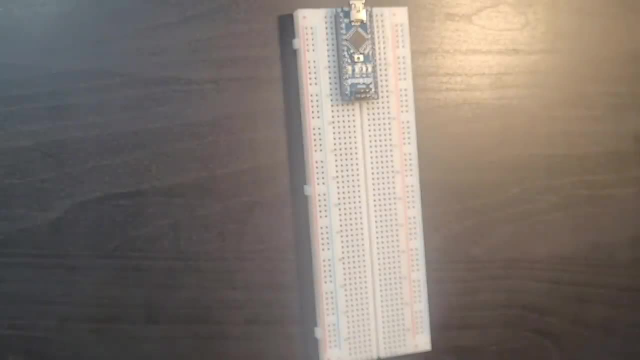 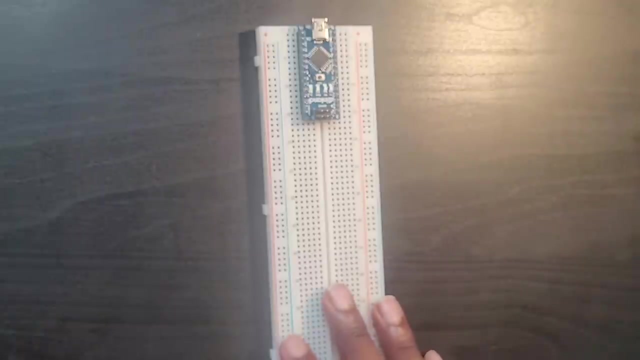 so, again, depending on the key you have, might have a different type of uh temperature sensor, but, uh, we're going to check two sensors, so we're going to see, we're going to check most of them, okay. so even then too, i'm going to show you guys how to actually see what type of sensor you have and 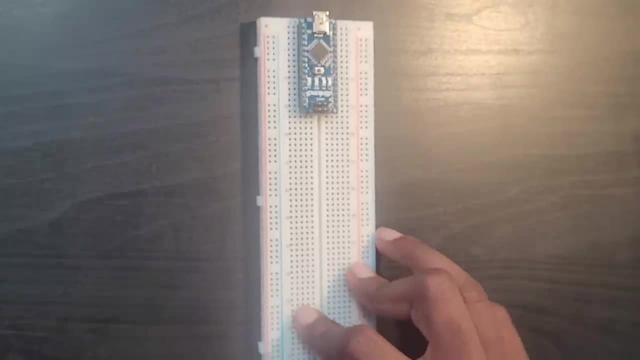 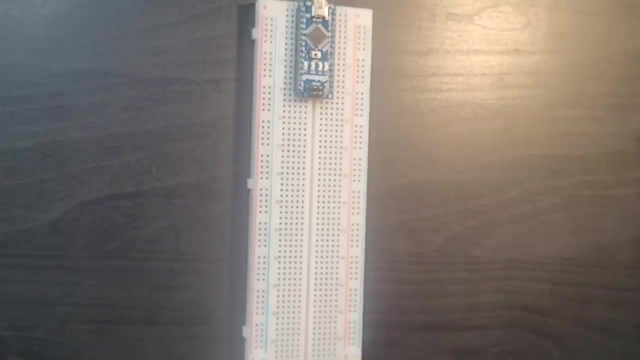 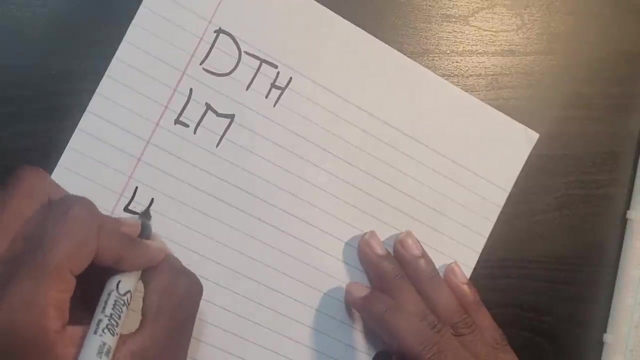 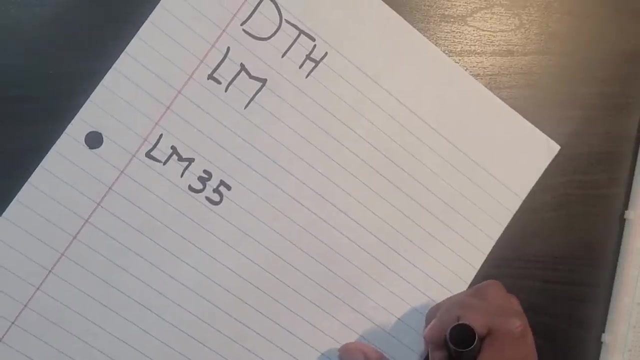 adjust accordingly to the sensor you have. okay, so, first things first. what i'm going to do is try to explain what these sensors are. okay, so let me go right here. the lm. right now, specifically, what i have is what? the lm sensors? the lm35, okay, the lm35 temperature sensors, but there's also one. 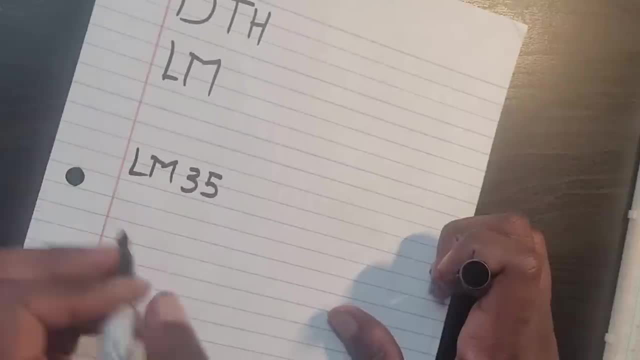 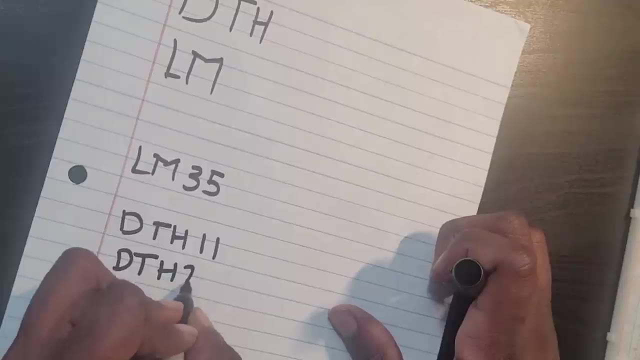 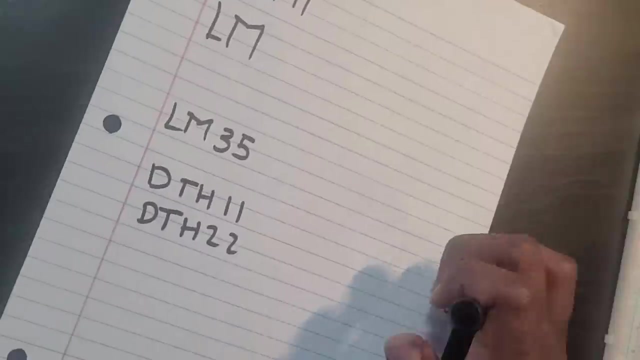 other common sensor, which is called the dth. there's like a dth series, the dth 11, for example. there's something called the dth 22, and these are one of the most popular sensor right here. so is this one, but i think this is far more popular. okay, so we're going to check how the 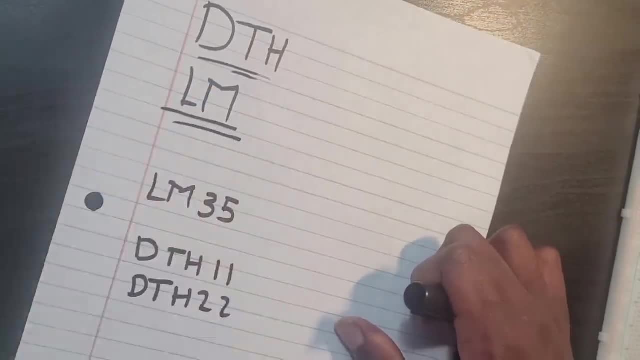 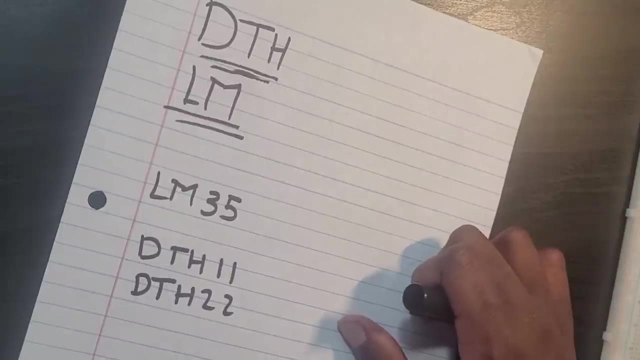 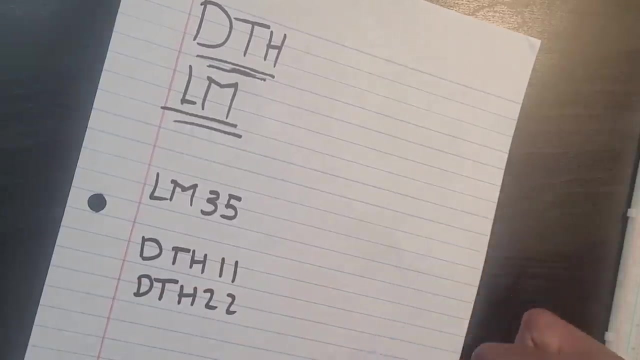 dth sensors and these lm35 lm sensors work okay. so if you don't have those type of sensors, i highly suggest that you guys watch a video of the sensor you have. first, know the sensor you have and then check a video, write the sensor's name and then check the video of uh, check a youtube video on it. okay, that's what i. 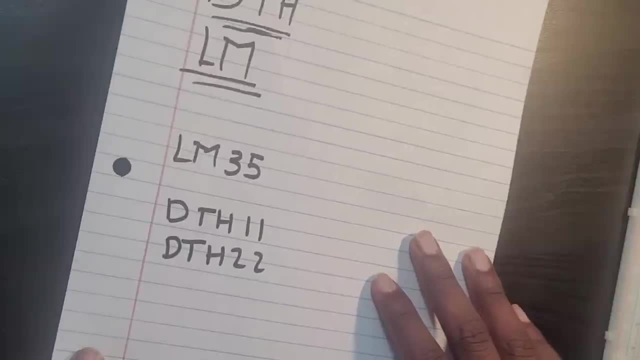 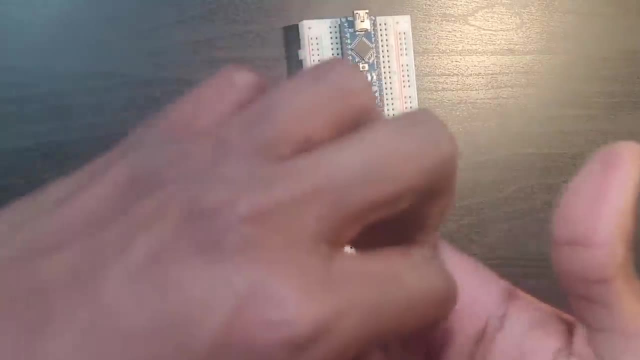 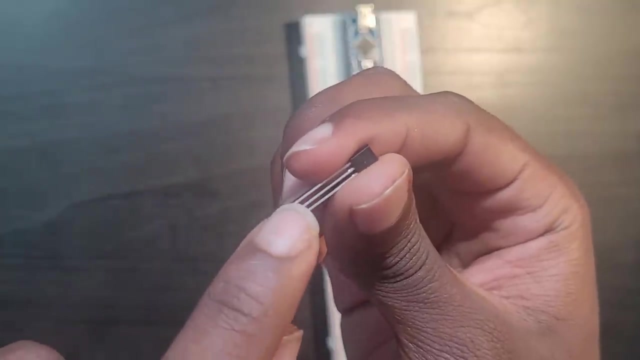 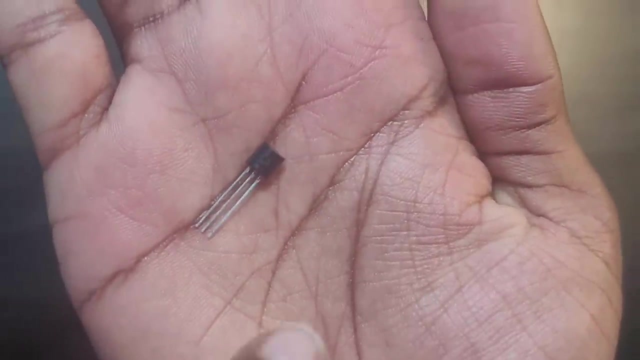 suggest before starting this temperature sensor, uh section. okay, so now what i'm gonna do is bring the sensor. okay, let me work with the lm35 right now. and the lm35- one thing you notice is what you know: this has three legs. okay, so we're going to put it where the text is. there's a, just produce it here. you can see a dot. 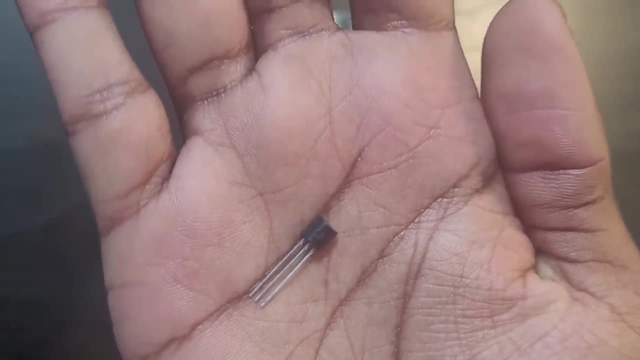 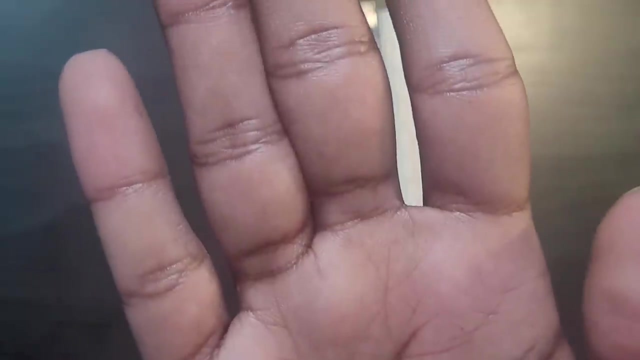 a black dot right here. not only that, too, but it's rounded. but we're going to go to the flat side, okay, the flat side of it, whereas there's where there is a text. we're going to connect it that way. so the the most left leg is going to be connected to the five volt, the middle one, and then we're going to connect the five volt to the mid one. 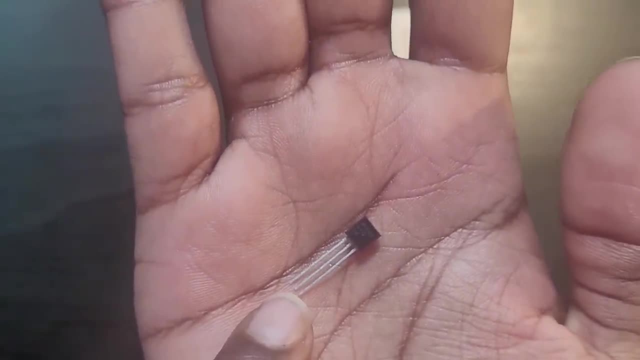 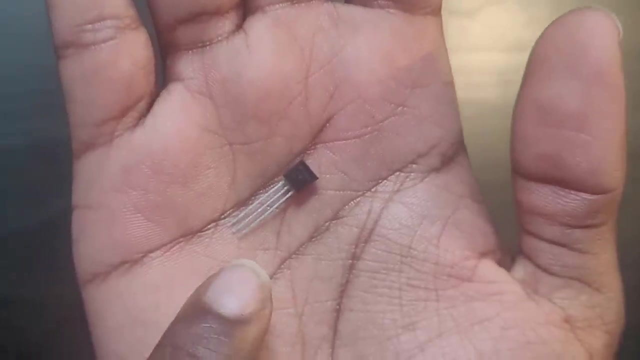 so the the most left leg is going to be connected to the five volt. the middle one, The middle leg, is going to be connected to the analog read volt- I'll get some analog volt again- And the right, the very right of this is going to be connected to the GND. 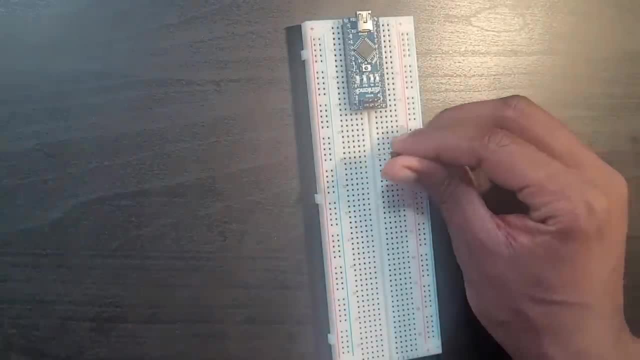 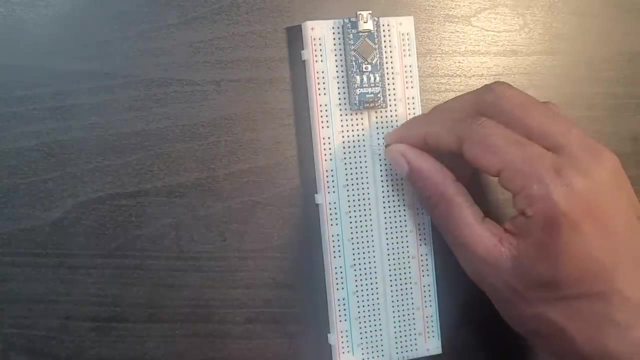 Okay, So let me just do that. I'm just going to put it right here. Just do that. Try to put it together. Let me just widen this a bit. I need to make this a bit wider. It's not going to fit in across. 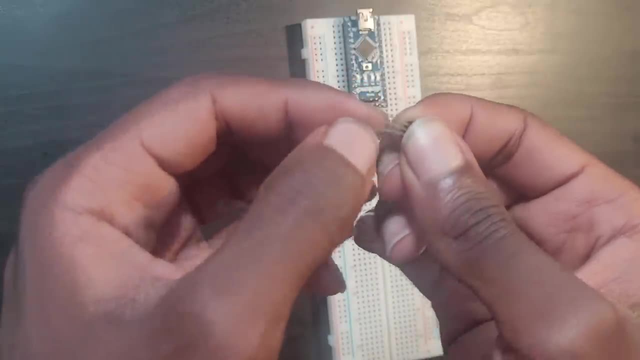 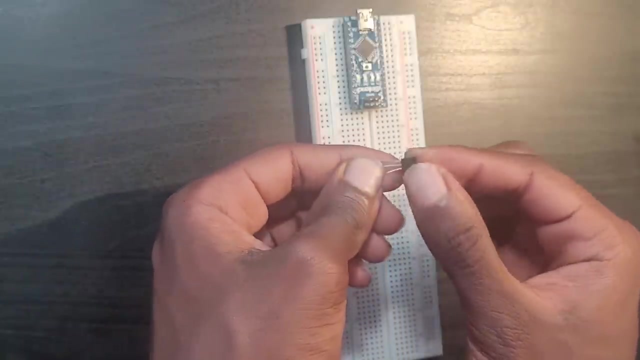 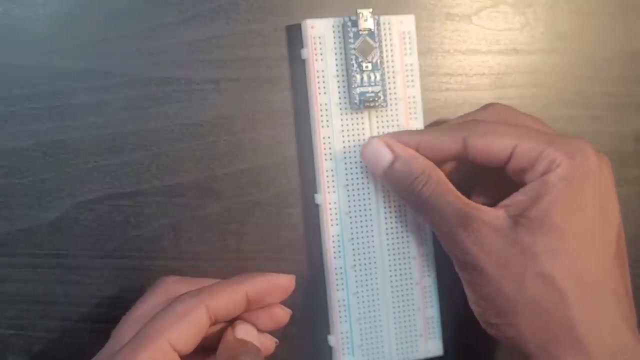 I want it to fit it across. So let me just make the legs a bit wider, Let me just bend them so that they fit. Okay, there we go, Thinking how they fit better, Okay, And come on, All right, Not the most, even one, but at least they fit. 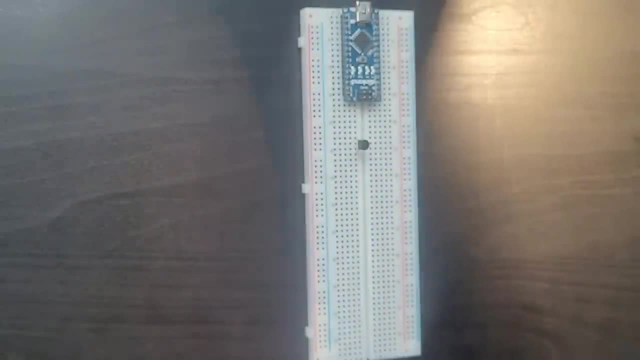 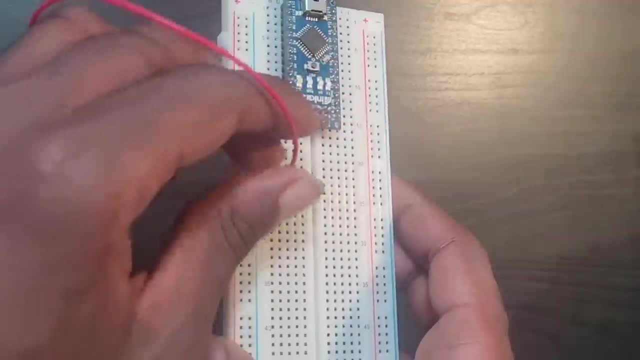 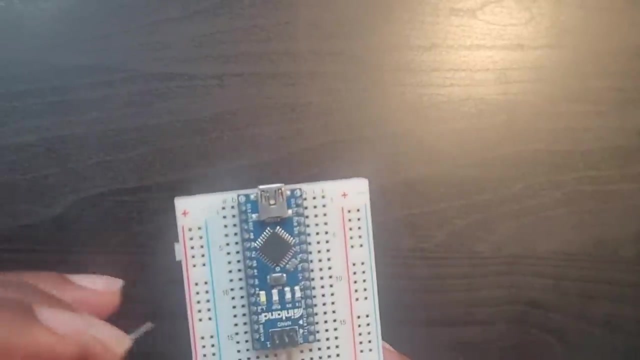 Okay, So what I'm going to do is connect again the 5 volt to the most left leg on the flat side. again, Let me just do that. The most left leg is going to be Connected to what's going to be connected to the right here. 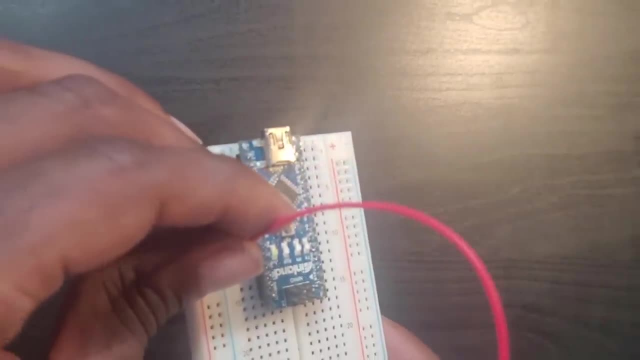 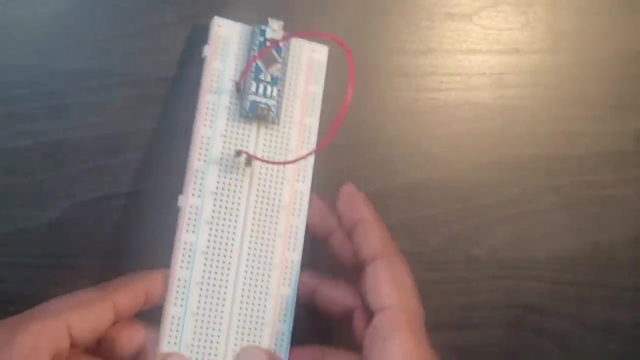 Going to be connected to the 5 volt. Okay, Let me just do that right here: Connect the 5 volt and the middle one. I'm going to be connecting it to what? To one analog pin that I left my choice again. 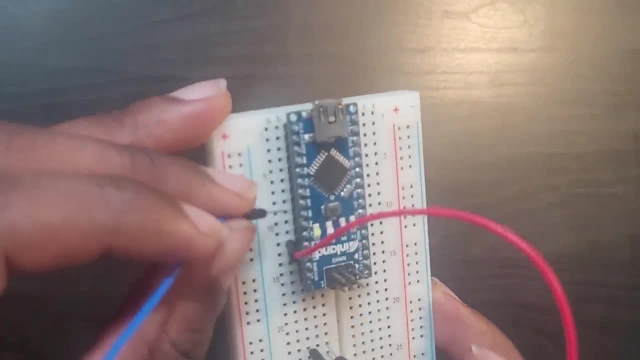 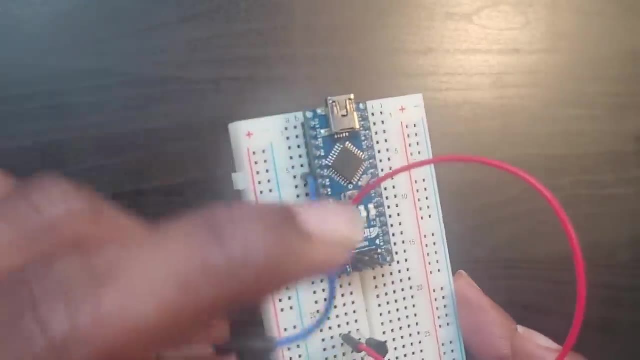 Let me just do that: Find an analog pin. I'm going to be using analog pin, maybe one today, Maybe an analog pin 2. actually, Let me just use an analog pin 2.. It's just a bit closer. I just don't want to stretch the wires. 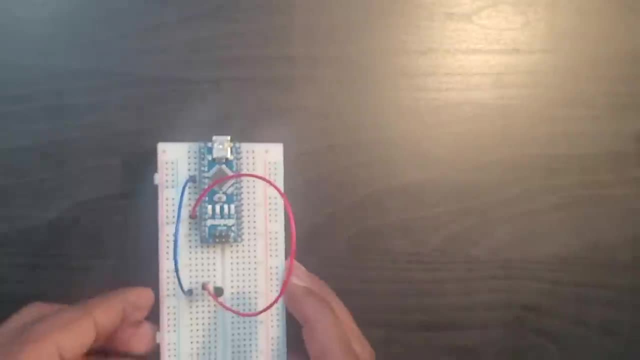 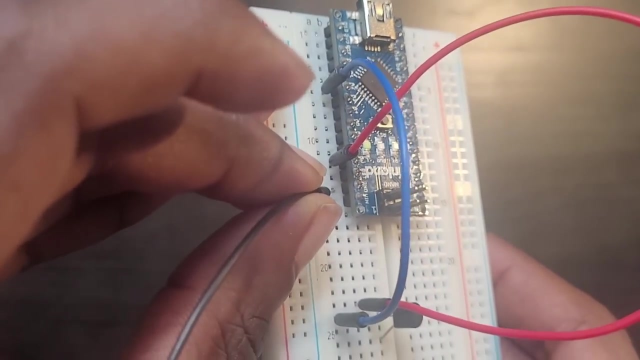 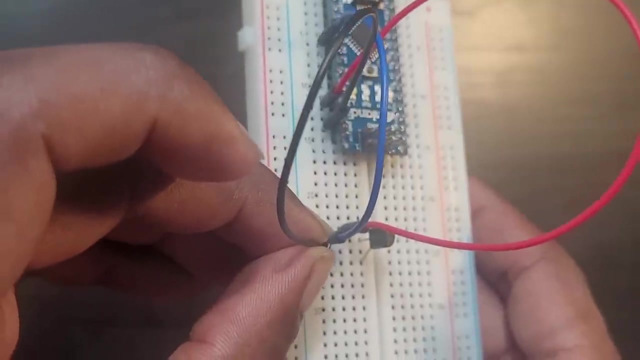 Okay, And then afterwards, what do I want to do? I want to use my GND pin. Let me just do that. Let me just go to my GND right here, Connect that to my GND. The ground. Let me just check if everything's intact. 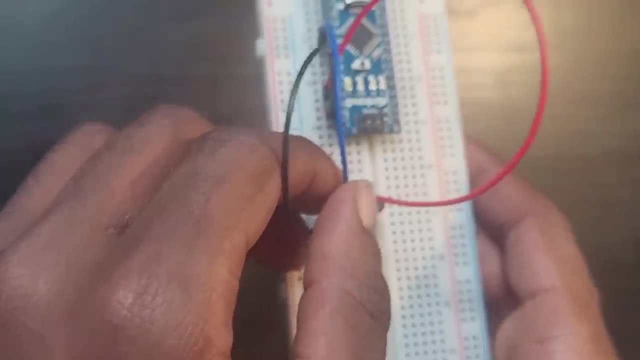 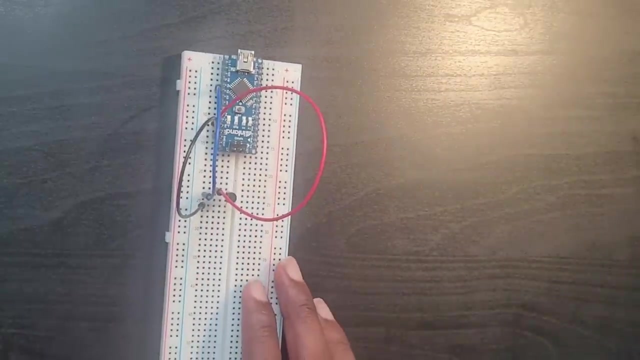 Okay, the GND is right here. Okay, Once I'm done doing that, what I'm going to do is write down the code. So let me go over to my screen right now and let's write a bit of code, Okay. 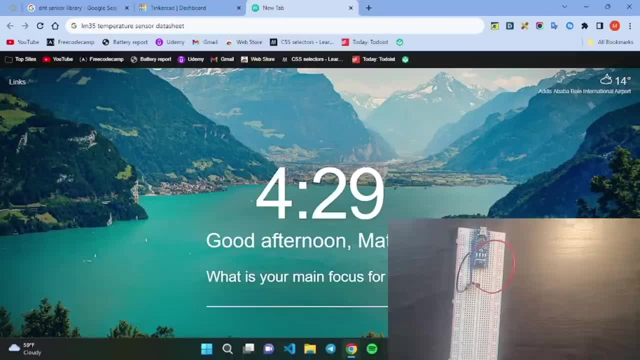 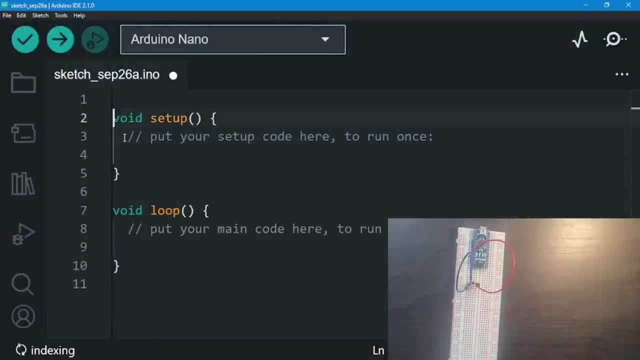 Okay, So let me open my Arduino IDE, Let's write one of this and let's set up our code. So, first things first, we need to set up what our read pin. Okay, Read pin is what today? Today is analog pin 2.. 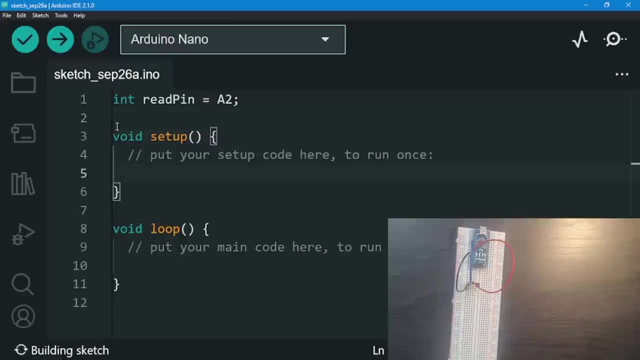 Now that 2.. Now, what I'm going to do is set it up right here in mode, Set it up as read pin And that is what, As an input? Okay, Because we're going to be what Reading from it. 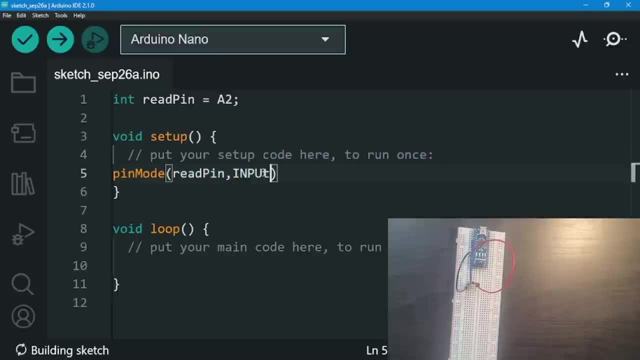 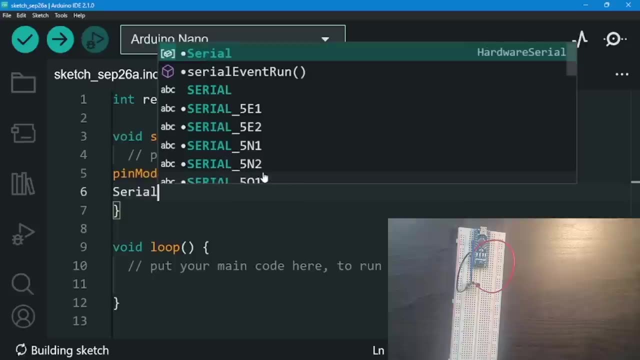 Okay Reading That T's not right. Let me just get that, and afterwards, what do I need to do? Start the serial monitor, because this is where we're going to see what We're going to see: the temperature Serialbegin. 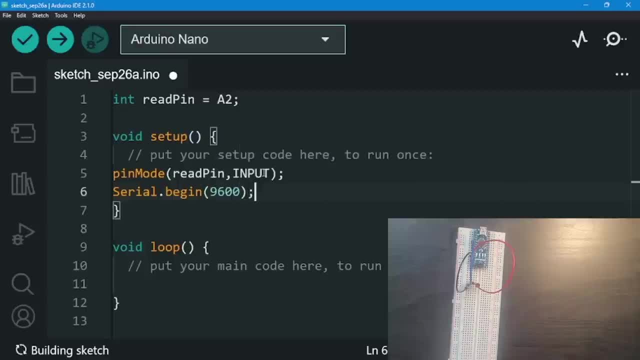 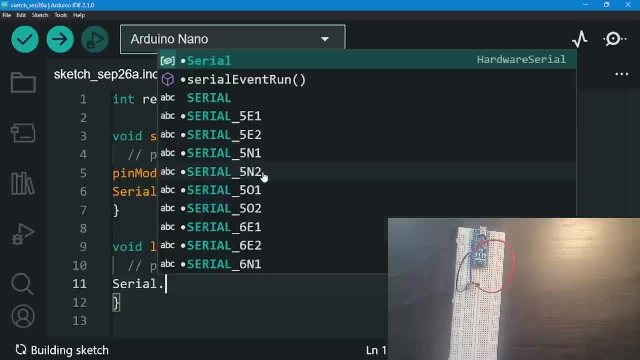 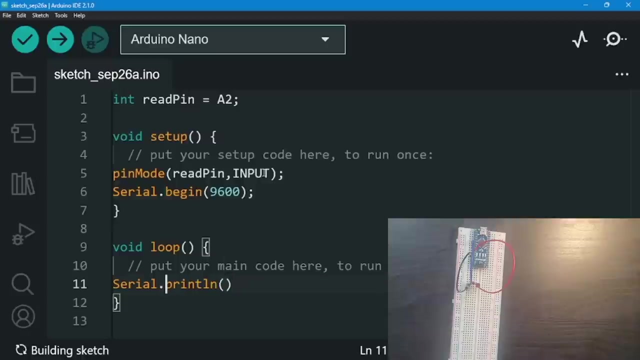 Again, with what baud rate? 9600 baud rate. There you go Afterwards. I'm just going to do serialprint. How the heck I'm going to what? I'm going to print a new line right here. With what? 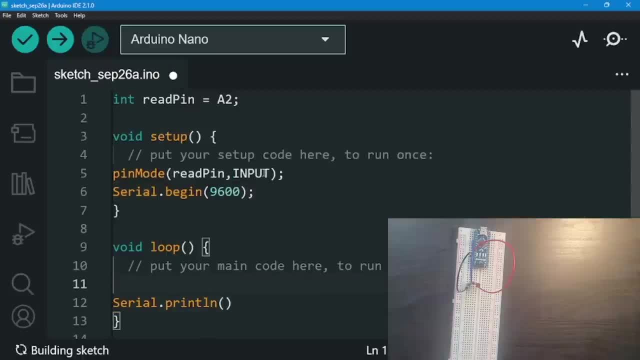 Maybe the read value First things first. do I need to do what I need to read? I need to analog read it. So analog read, All right. So obviously this is not making sense. I'm just trying to read the value. 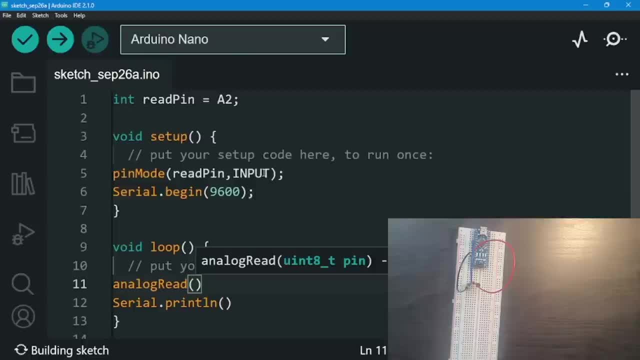 But what we're going to do is, first is what Change the red value to what? To voltage first, And then we're going to go to check the math and how to change it to Celsius. All right, So let me go to analog read. 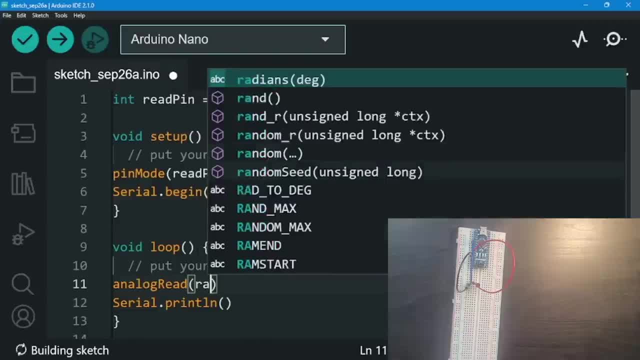 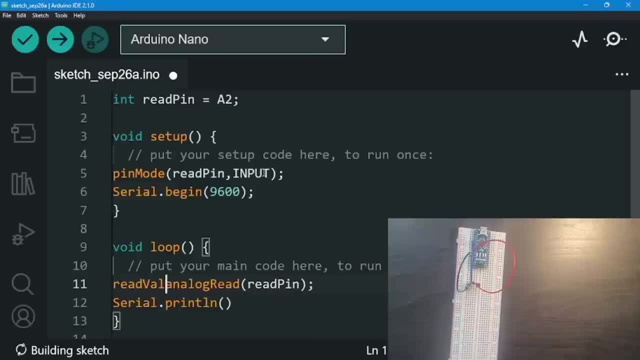 In this case, it's going to be what Analog read, the read pin. This is going to be what This is going to be: The read, The read value. It's going to be the value that I'm going to read, which is set like this: 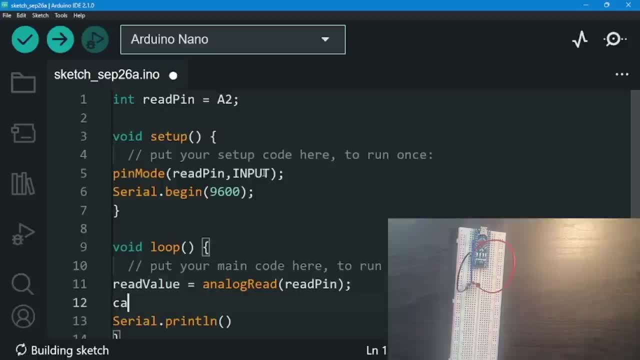 All right, And afterwards, what? Then? afterwards, we want to say: calculator value, Calculator value is what? The read value? You've got to divide it by what? 10 to anything. I'm going to, Actually, we're going to multiply it by what? 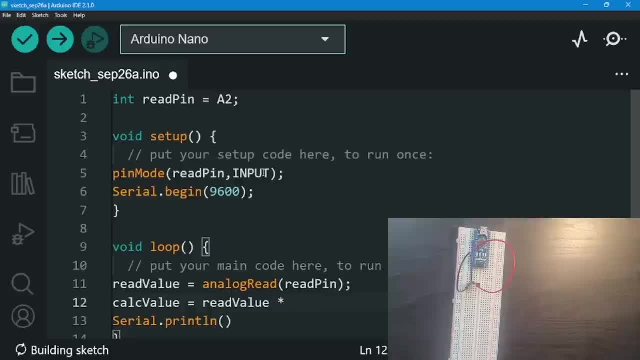 Let's do a five point right here. Again, you know why I put five. You can also put zero right here, because it's going to be a flow. I don't want it to what Round, Round, Up or down Round. 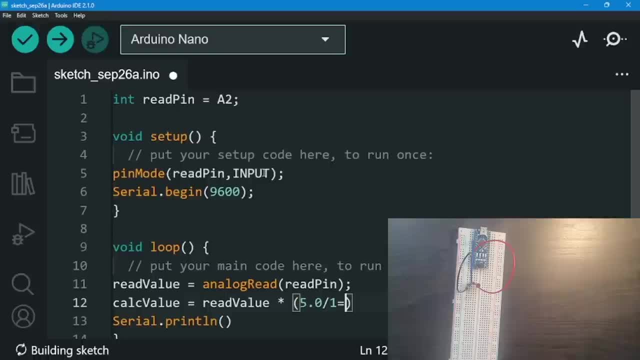 Round, Round, Round, Round, Round, Round Up or down After it's done calculating it, because then it's going to be a zero. Okay, Five point. Oh, we're 1023.. I can add a zero right here, or not? 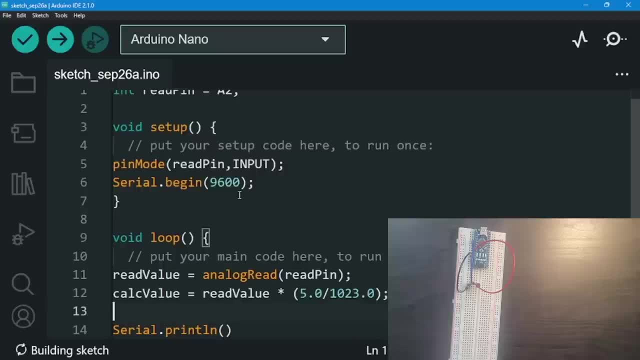 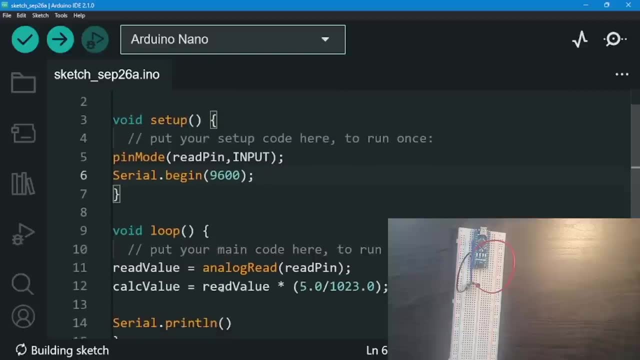 It's up to you. Okay, Then, once I'm done with this, what I'm going to need to do is go right here. Okay, There's the calc value, Calculator value. Okay, So the change is degrees Celsius. first, What I'm going to need to do is go to my browser right here. 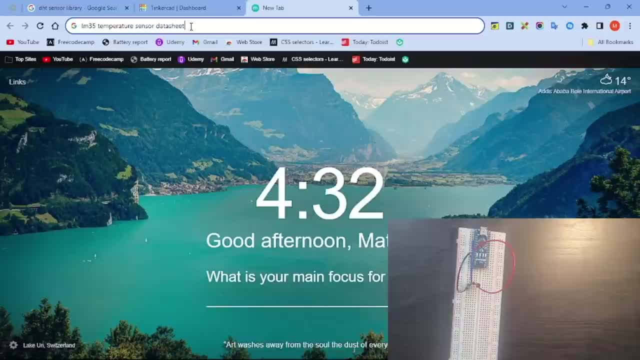 And I want to. What I'm going to need you to do is: most people have an LN35, by the way. Right, They're going to be following me in this section. If you have a DHD sensors, I'm going to come back to them and actually show you in the 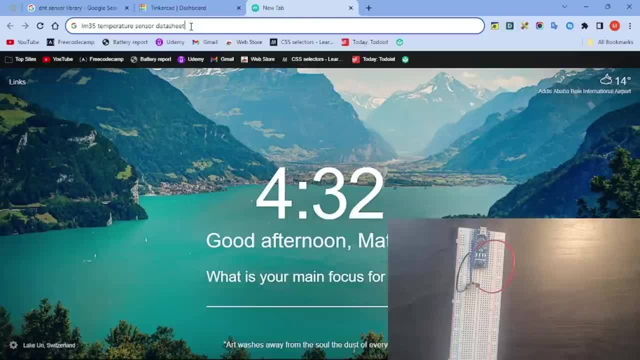 next section. Okay, So for those who only have LN35, we're going to proceed If you don't have a DHD or have another type of sensor again, if you have another type of sensor again. watch another YouTube video. 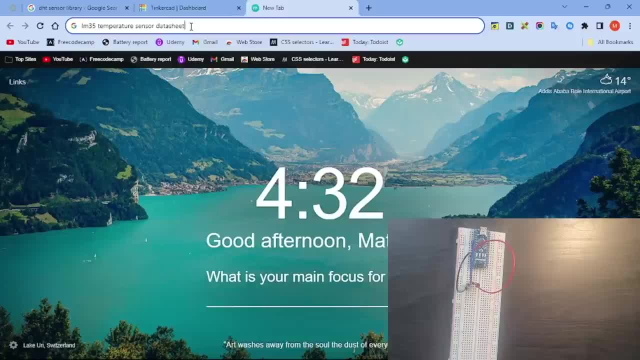 There are lots of YouTube videos to get of any sensor that you really need. You're going to find lots and lots of resources, But if you're using a DHD, hang on Wait. Skip to the next section And I'm going to show you how it's done. 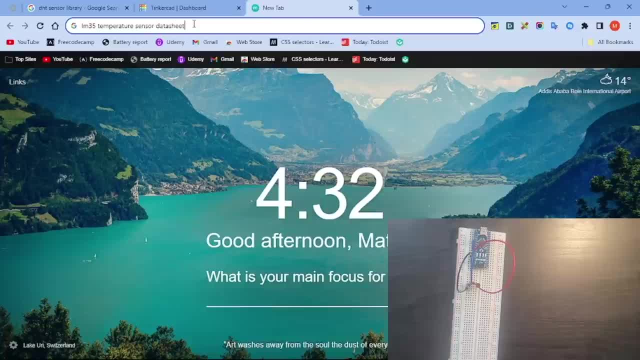 Okay, So when it comes to the LN35 temperature sensor, we're going to go to its data sheet. I want you to search this: for what? LN? and the corresponding number Right now, at 35.. Temperature Sensor, And go to data sheet. 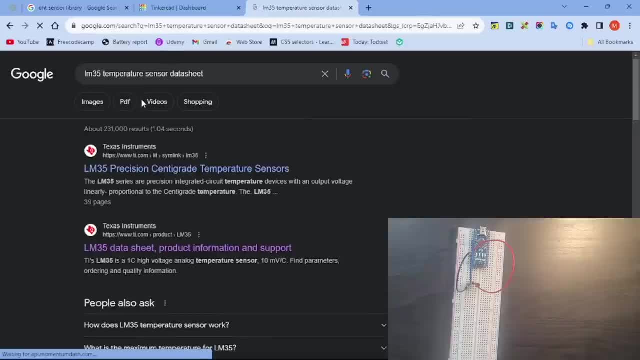 All right, Let me just do that And you're going to find some sort of PDF around Precision centigrade information and support. I'm just going to go over here. Oh, actually the PDF is right here. It says 39 pages here. 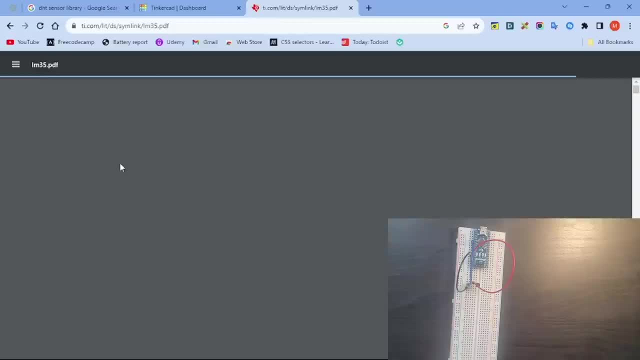 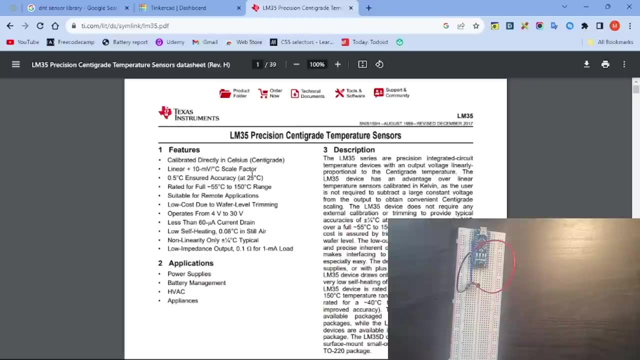 So let me go here to the PDF. All right, And on this PDF right now, the documentation of the LN35 you're going to see is what The description and the features it has It's going to measure, to what It can measure. 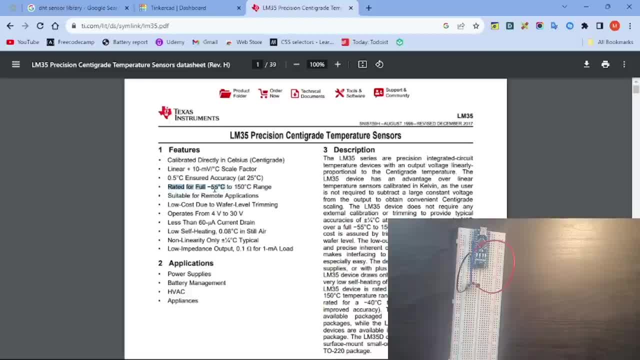 Look at it: The rate of airflow from negative 55 degrees Celsius to 150 degrees Celsius. This is what The temperature range. All right, The range of temperature is what? From negative 55. To 150 degrees Celsius, So it can go a lot. 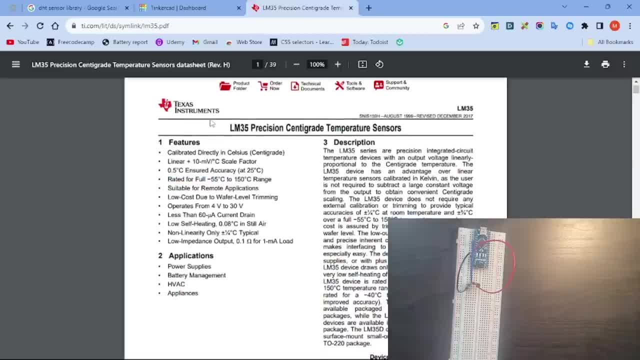 Okay, Again, this is going to be different for the type of LN that you have. I have an LN35.. Okay, So, once you're done with that, reading this- And, by the way, there are lots, I'm talking- 69 pages of documentation. 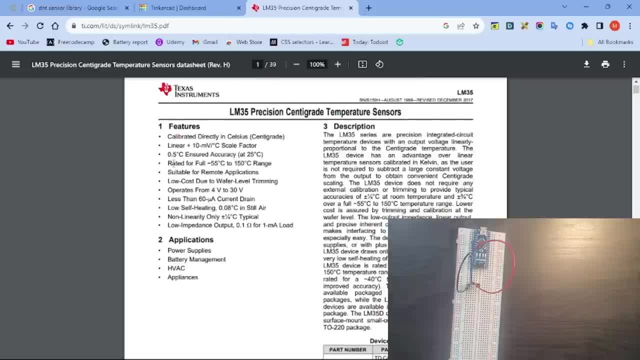 But we're not going to get into any of these because they're advanced All right And you don't need them in this case. But again, any information that you're going to need, you can find it here in the documentation, In the official documentation of what. 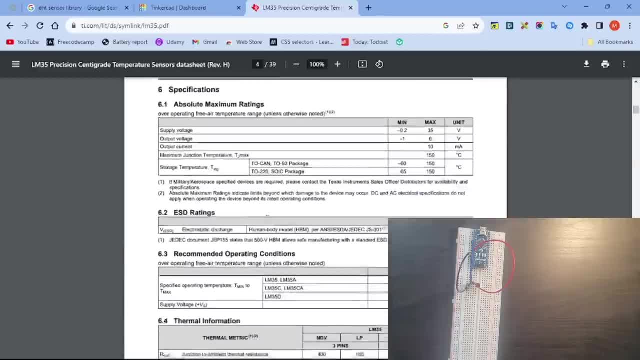 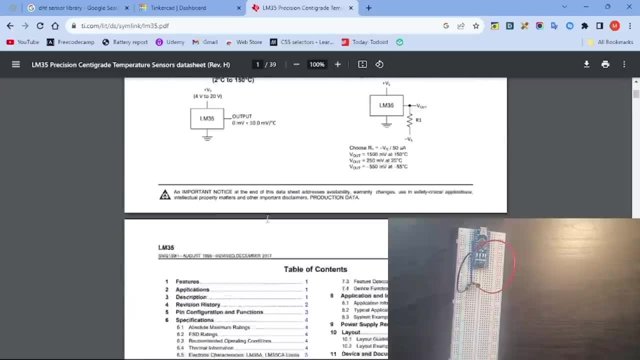 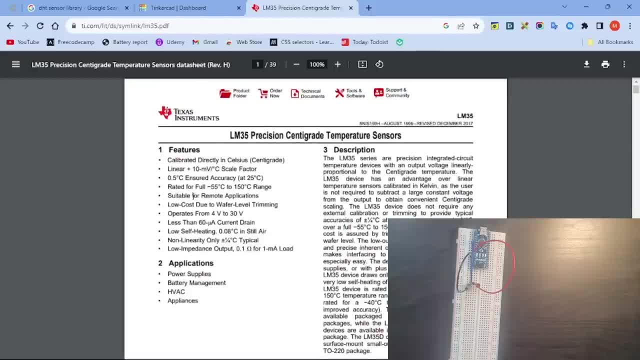 The temperature sensor. Okay, So one thing that you should focus here is right here. you should focus at this one And the highlighted. There we go. This one: It sees linear plus 10 millivolt per degree Celsius scale factor. 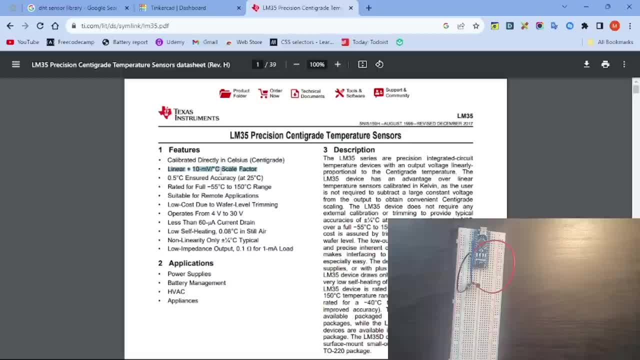 So what does it mean? It's saying that the scale factor basically is what It's going to, what It's going to output: 10 millivolt per every degree Celsius. Okay, celsius, all right. so for every degree celsius that, um, it monitors again. it's going to what sense? 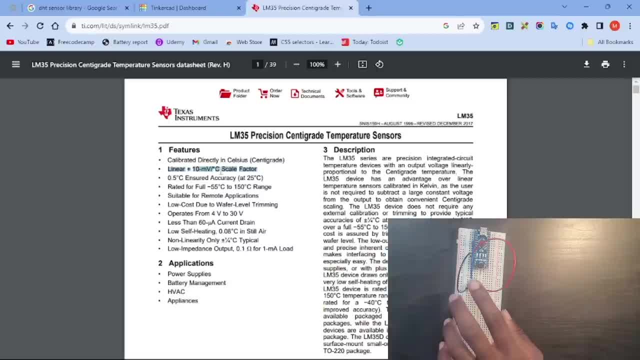 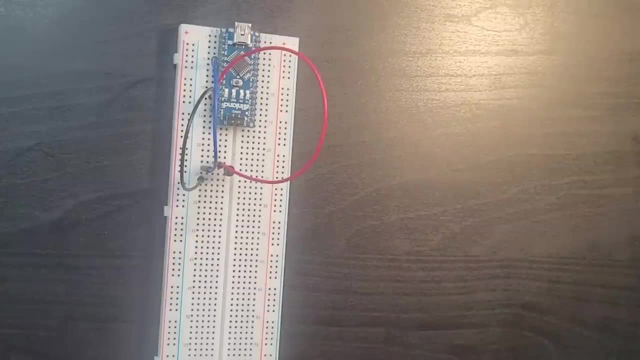 it's going to apple. what for for analog pin in the middle, the blue pin, the blue wire, it's going to be outputting with 10 millivolts. okay, so it's going to be outputting 10 millivolts, okay. so right here, let me just bring my paper right here, paper, and let me do the sharpie and let's try to. 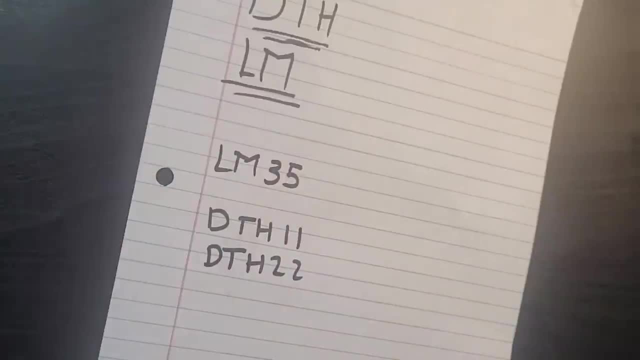 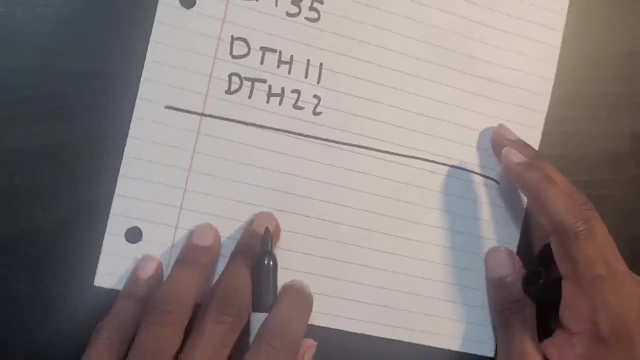 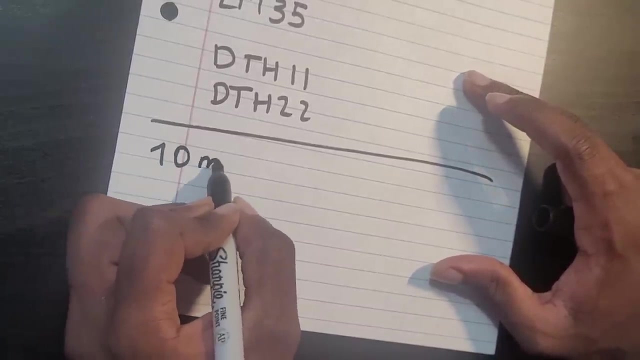 understand what that means. let me just put this out here for now, okay. so let me just draw a line right here and let's focus on this line on the space, okay. so what does this basically mean? 10 millivolts per degree celsius. let me just write this down: it means 10 milli volt. 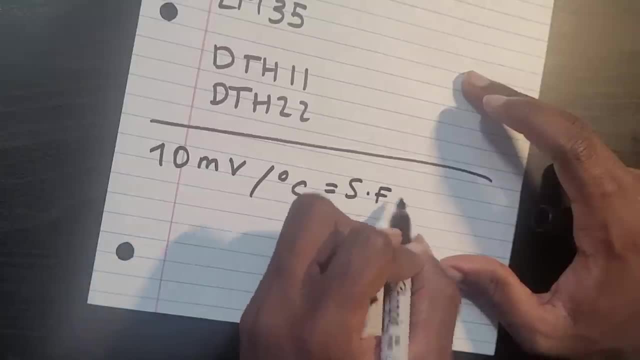 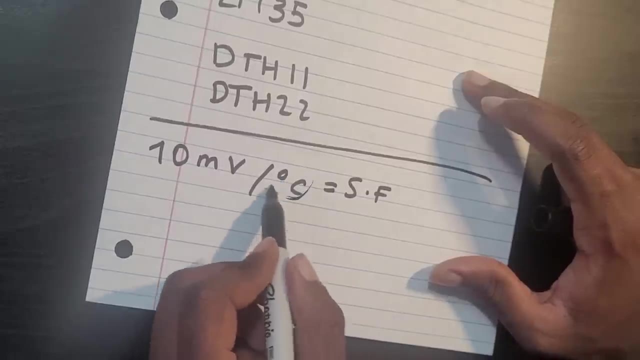 per degree celsius is what the scale factor. okay, i want you to focus on this. what do we want to get? we want to apple. what we want to print the, what the temperature we want to put, print the temperature. so what does this mean? 10 millivolts means what milli? 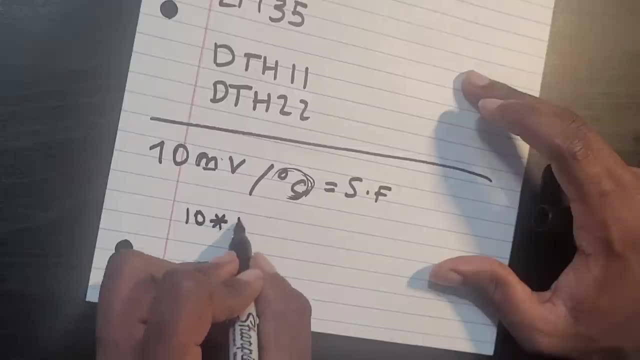 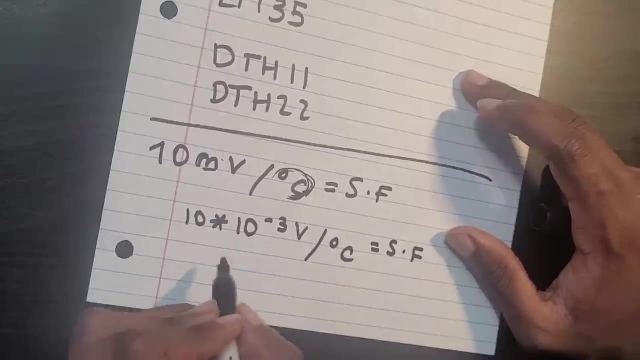 stands for 10, the power of minus 3, so which means 10 times 10 to the power of minus 3 volt per degree celsius is the scale factor, which means if you multiply this, this becomes 0.01 volt per degree celsius. is what the scale factor. all right, so what is scale factor? 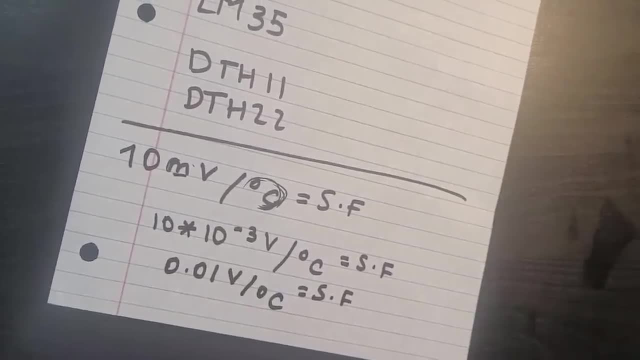 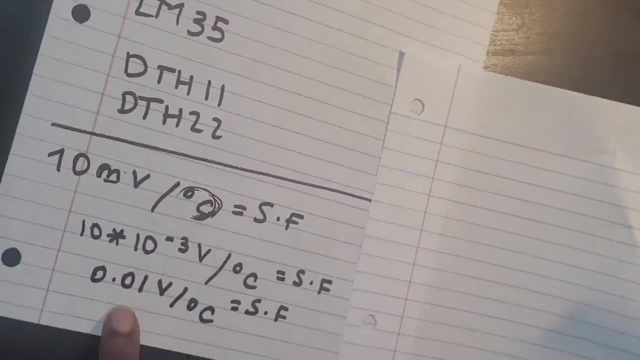 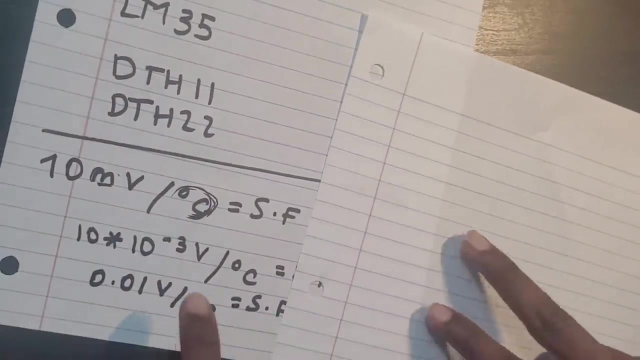 right here, let me just bring another paper. okay, let me just do that. i'm running out of paper. right here, just bring another one. so what does the 0.01 volt per degree celsius mean? okay, you said this is what the scale factor. again, scale factor is what voltage over. 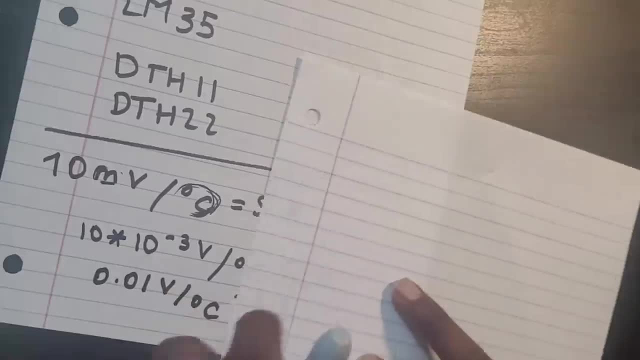 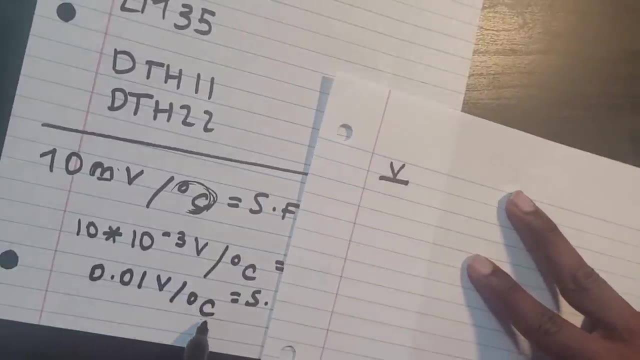 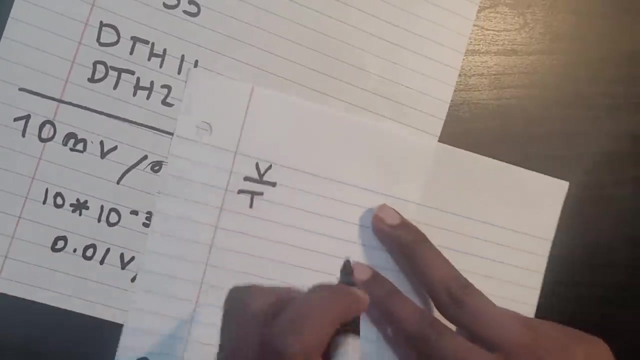 temperature. you can see their units. what is the unit of volt voltage? so what does this mean? volt over. what's the unit of degree celsius? what is the? what do we? what is the unit of degree celsius? um sorry, degree celsius is the unit of what? it's the unit of temperature, okay, and this means v over. 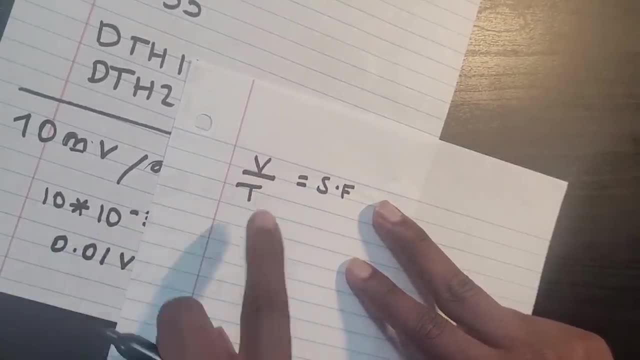 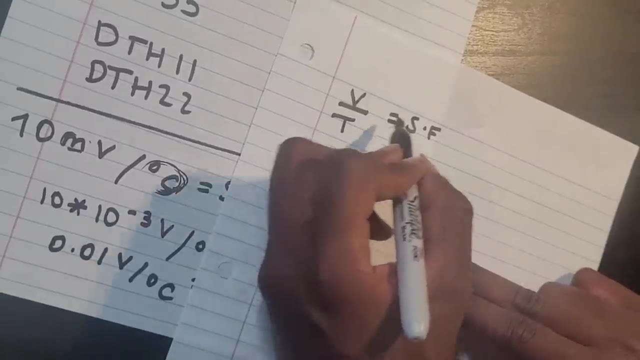 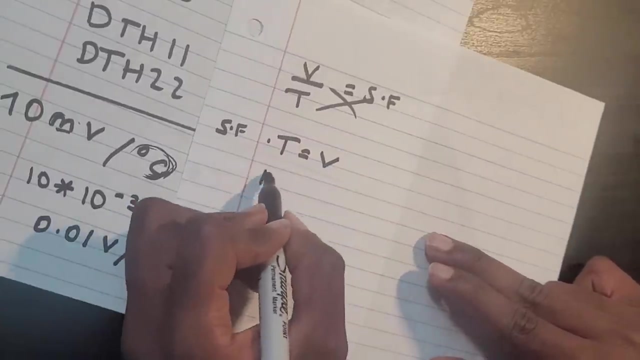 t is what the scale factor. it means voltage over temperature. trying to find what temperature again, keep that in mind, okay. so temperature is basically what the scale factor. so let's do a crisscross: temperature times the scale factor. in this case it's going to be what the voltage. all right, so 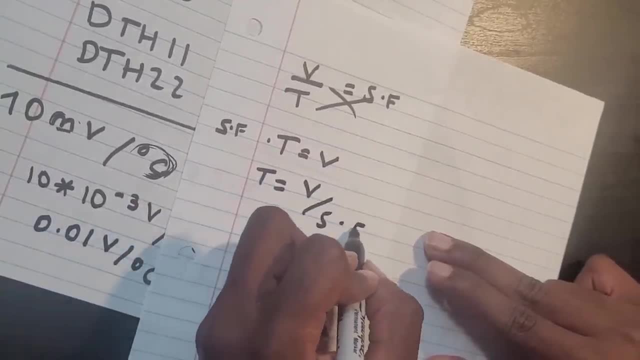 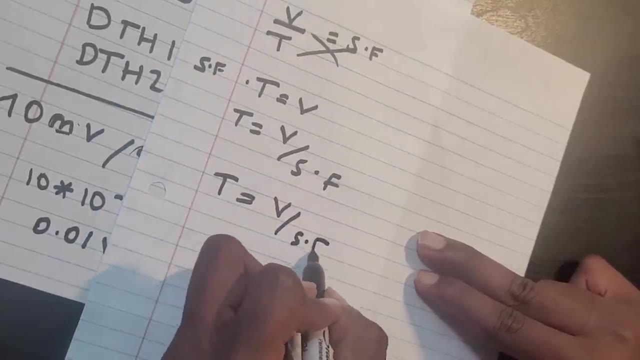 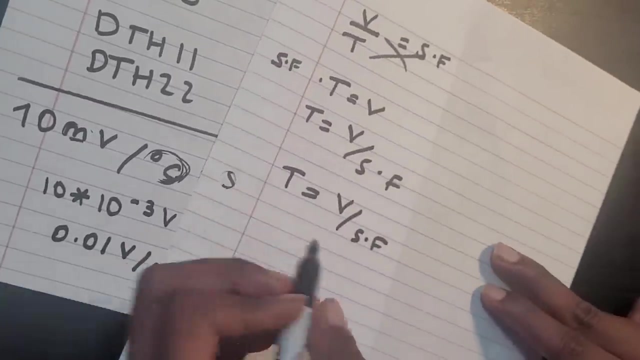 we're going to divide both sides by the scale factor. okay, then temperature. temperature is going to be v over sf again. what is sf? sf is what? 0.01 volt per degree celsius. the value is what? without the unit again, if we just do the unit, it's 0.01. okay, that's one thing. 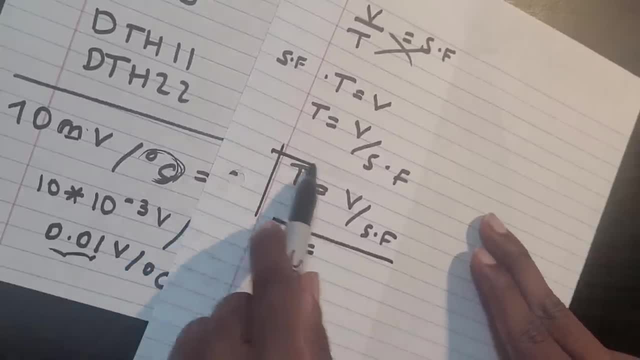 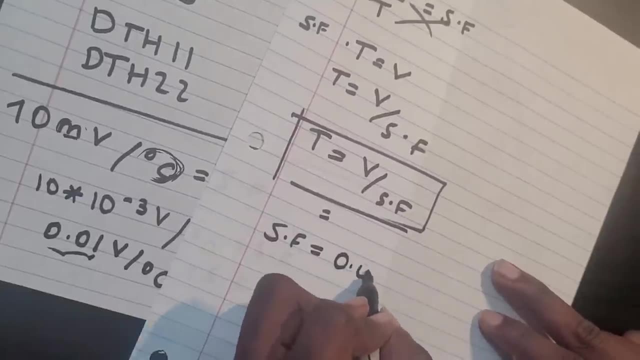 i want you to keep in mind these two: temperature is what volt over scale factor and scale factor is what? the value of scale factor is what? zero point zero one volt per degree celsius. 0.01 volt per degree celsius. why did we need to change from millivolt to volt? 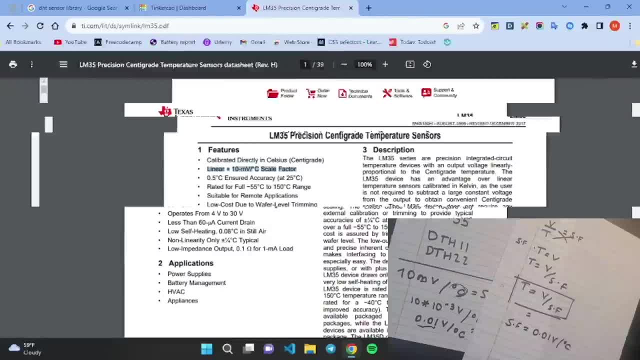 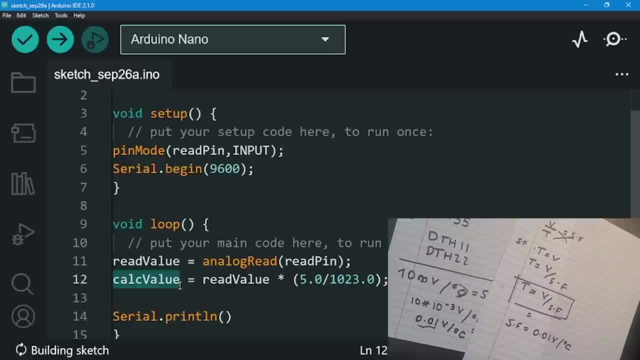 because, as i said again, let me go over again to my screen- because our calc value is going to output what our calc value is going to output, and volt, not in millivolt. that's why i have to change the standard from millivolt to volt. all right, 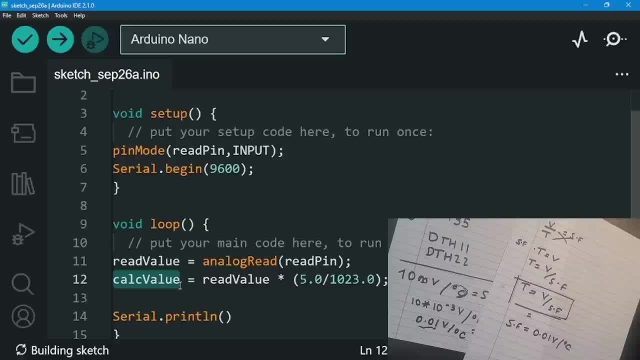 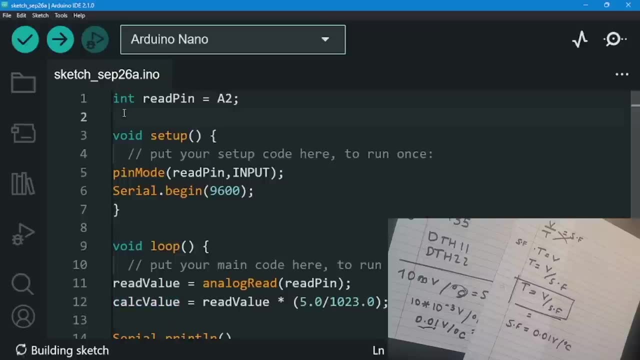 because our cap value, our calc value, is going to output in what and voltage and v. okay, so what are we going to do right here? so we're going to need to set up what we're going to need to set up, uh, the, what, the scale factor. so what i'm going to say is here: 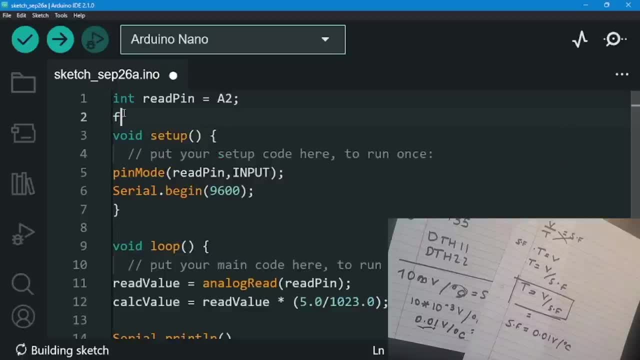 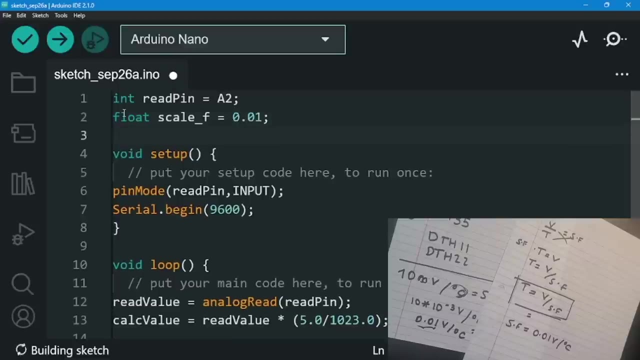 um int scale factor? actually not, and it's a float, float. i'm just going to say scale. i make this very short scale f. it's going to be what? it's going to be set to 0.01, all right. and then i'm going to need what temperature? i'm going to say temperature, i'm not going to set it up yet. 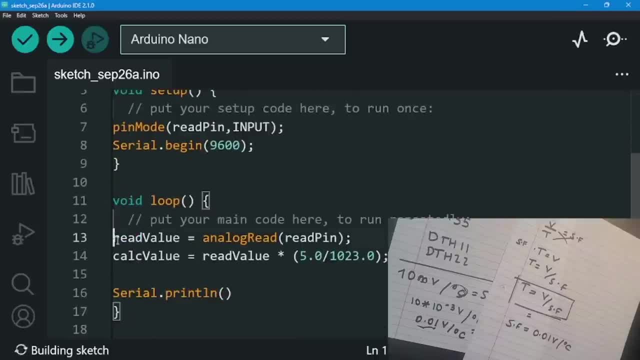 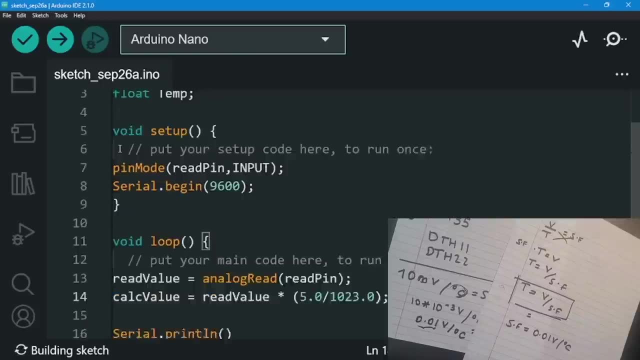 then we already have calc value. i do not set up calc value and read value right here. as you can see my code, i have to set it up right here. i didn't do that. so that's always what recommended: to set variables first, and then what, and then assign them. you can do the opposite way again. 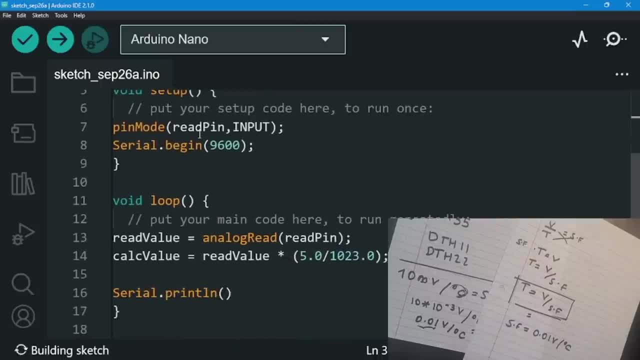 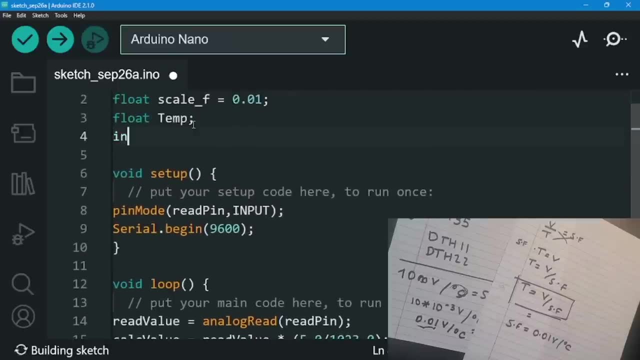 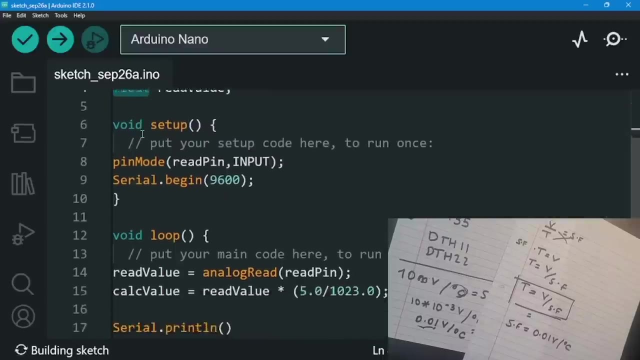 sometimes you might forget about what you might forget about setting it up. so i already set up, uh, float and temp. so let me just go right here and set up read value. so i'm going to say float, read value, say float or int. in this case, read value is going to give me a number between 0 and 1023. 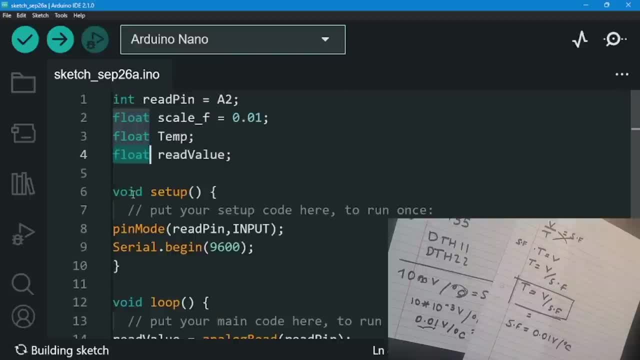 it's not going to give me what a float number. so obviously in this case i can say float or i can say hint, it doesn't really matter, but i can say end. right here. it's again makes sense for me to see it. okay, so you can see int or float, but i'm going to again say float because i'm going 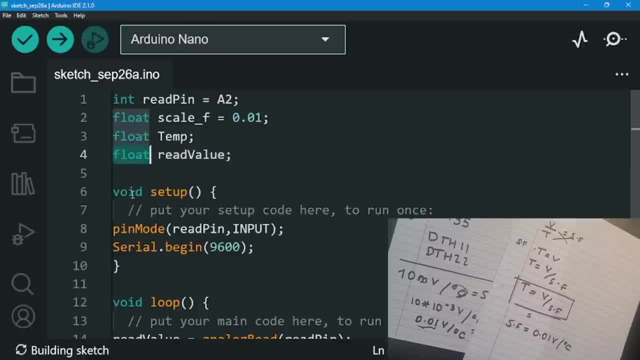 to be multiplying this and working with this. so it's suggested that you say float, because you don't have to think about it. when you say float, you have to think about. let's say it. okay, in this case, read value outputs: 10, 23. okay, if it's an integer, it's going to operate as 1023. okay, if it's a float, it's going to operate as. 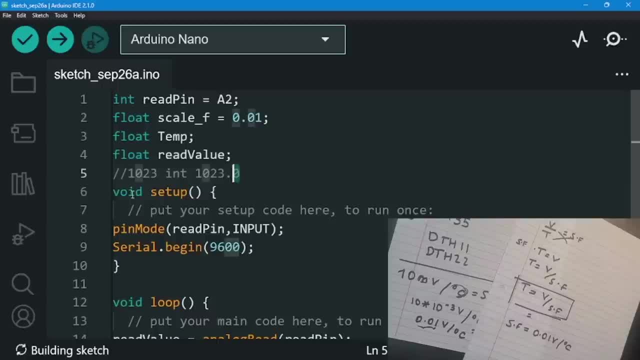 what this is going to put it as 1033.0, which is exactly the same thing, because a float, it's going to output it like that, which is exactly the same thing. so when you say float, you don't have to think about the most things, you have to think about them. okay, so you can just say float and 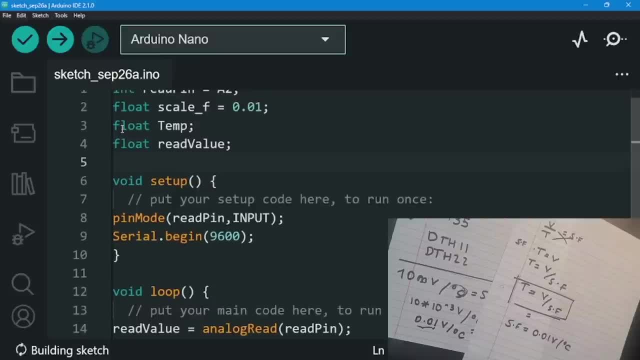 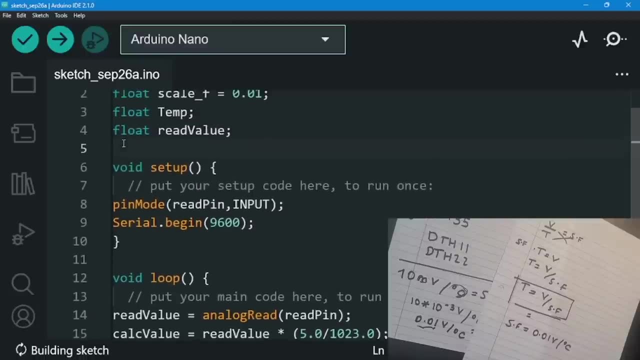 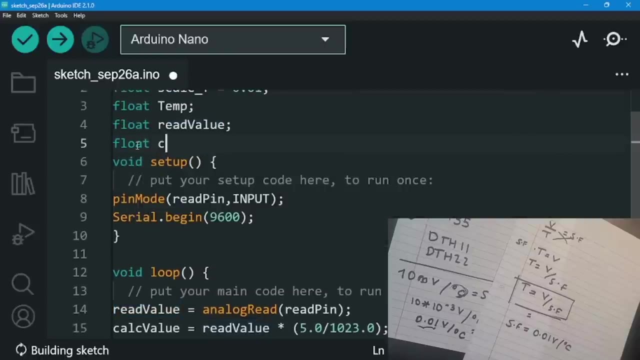 just not think about you know it, um it, uh, about it being an integer or not. you can just use float for everything, okay, so after using that, what i'm going to need to do is, after i'm done with my read value, okay, i'm going to need float calc value. now i need the float value because i'm going to be 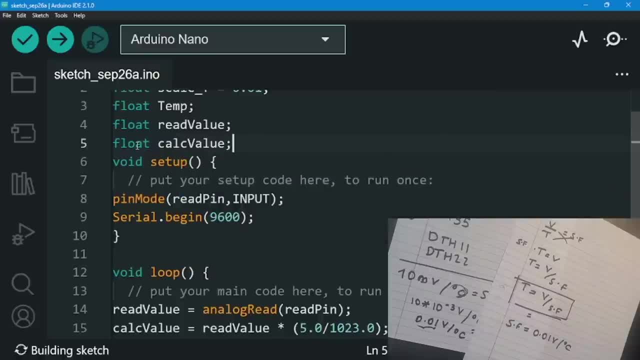 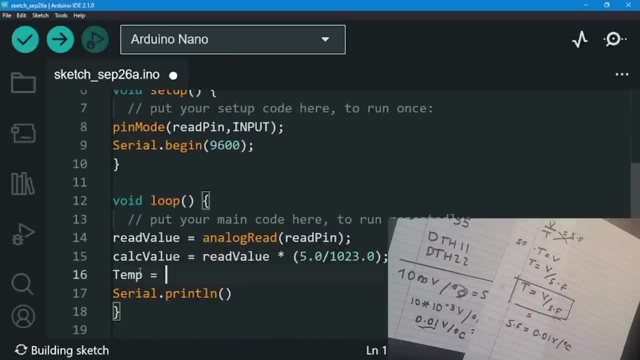 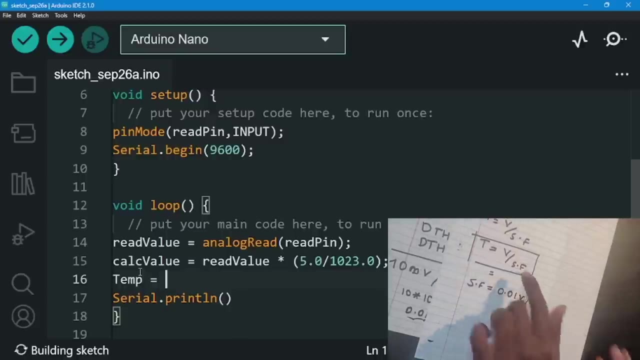 multiplying and dividing right, float calc value. let me just set that up. okay, once i'm done setting that up, temperature is what. as we said again, temperature is what temperature is what temperature. let me just go again, point here: voltage over what scale factor? sorry, voltage is what? the value that 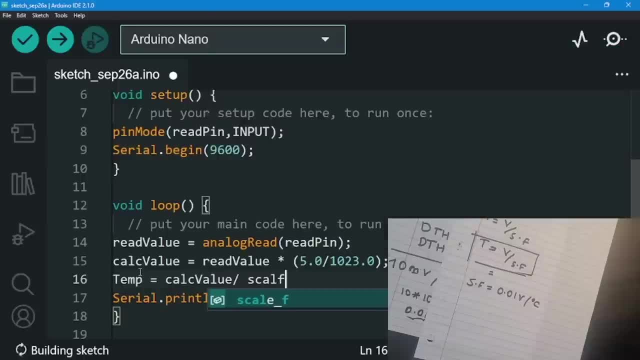 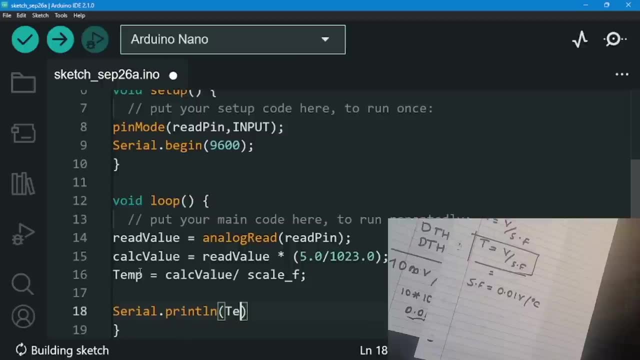 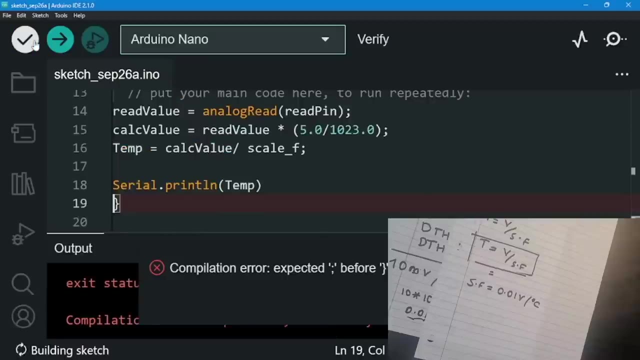 we're going to be receiving right here over the scale factor. it's going to be s scale underscore f. okay, so let's print the temperature right here. let's print the temperature. let's just do that. let me just first check. even if our code is right, it's saying that i'm not put a semicolon, i have. 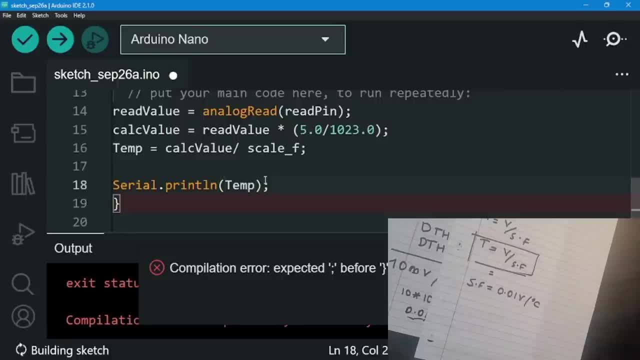 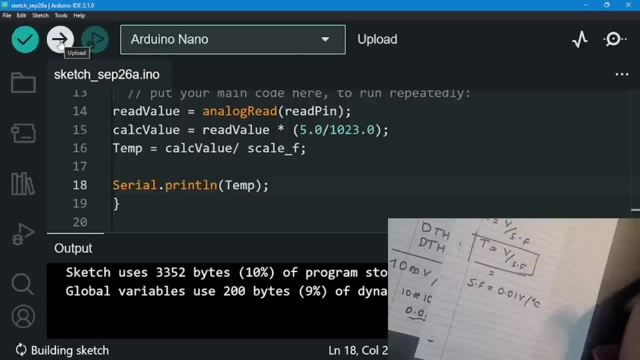 to put a semicolon after every what, after every line code. let me just do that and okay, it's done compiling and first thing i need to do is what? connect my arduino. i don't want to do that. okay, let me just do that. let me just bring that right here and connect my arduino. just forgot to do that. okay, now i. 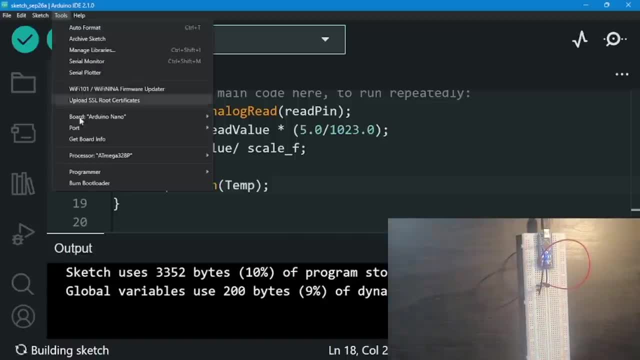 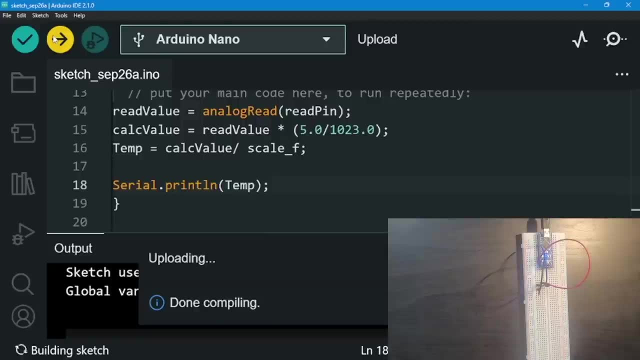 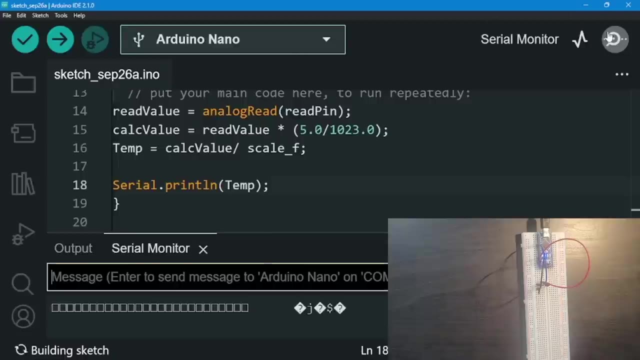 can upload, hopefully. let me check if it's connected. it should be showing me my port. okay, let me just select the port and let's upload it. it's uploading and it's still uploading. okay, we're receiving numbers very, very fast, so one thing i'm going to do right here is give it. 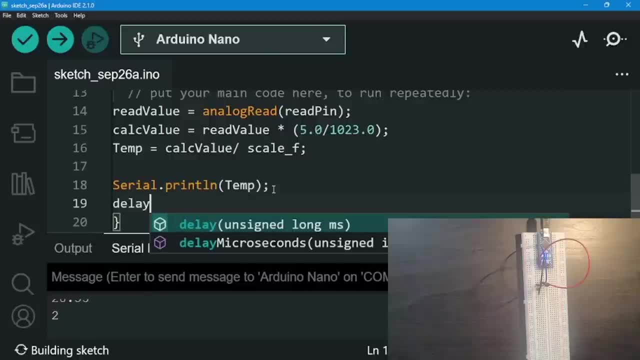 a delay. i forgot to give it a delay because it's going very, very fast. i can't even read it. we go delay and let's set it for 100 milliseconds. 100 milliseconds, actually, what? let's do 250 because it's going to be really fast. i don't want it to just go really, really fast. 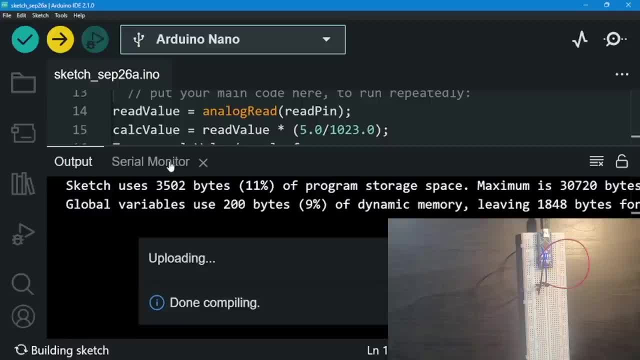 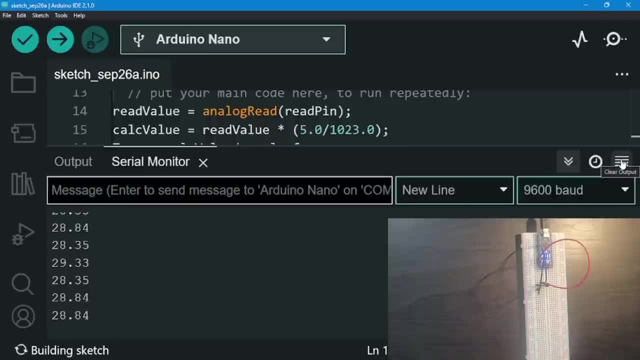 i'm just going to open my cylinder right here, it's going to open itself. okay, let it clear out. let me just clear this out and just say: clear output. and then it should be giving me an output, just 28. so it's saying that i have what? 28.35 degrees celsius. 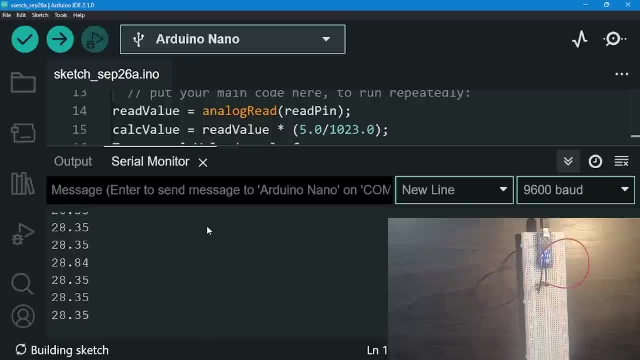 by the way, for this, if you are thinking you know what? why are we getting 28.8, three, five? how am i supposed to change this to fahrenheit or everything? why did i wait? why is it specifically degree celsius? why is that so again, let me go to documentation. it says what. 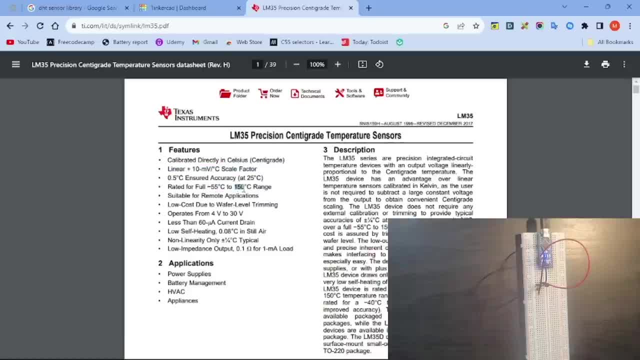 from negative 55 degrees celsius 250 degrees celsius. and, the most important part, what it's saying, 10 millivolt per degree celsius. right, it's saying 10 millivolt per degree celsius. what scale factor? so, basically, what we're using, the, what, the unit celsius. that's why i'm exactly sure that it's. 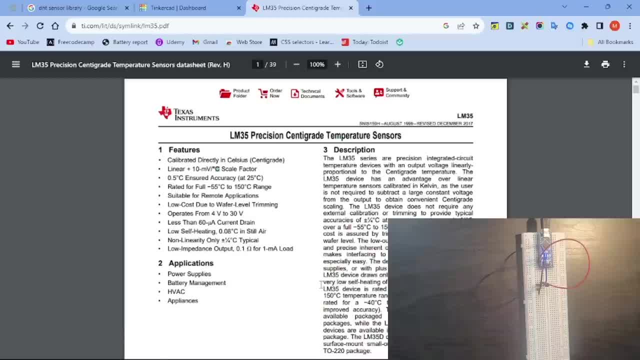 using one degree celsius, all right. so if you want to change it to degree fahrenheit, all you need to do- by the way, let this be homework for you- so what i want you to do is pause this, uh, this course right now. pause it right now. and i wanted you to do is change the degree celsius to fahrenheit. we already 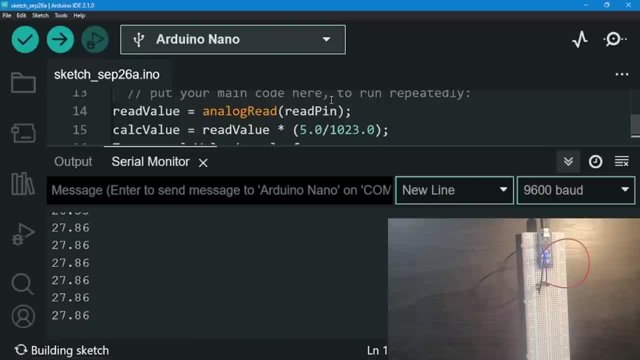 gave you the degree celsius right here, which is going to be- uh, it's going to be temp, tmp, temp. i want you to do what i want. i want you to convert it to fahrenheit. okay, so pause the video and do it right now. and i'm just going to do it right now. so pause the video, all right. so i think you, you've done it. 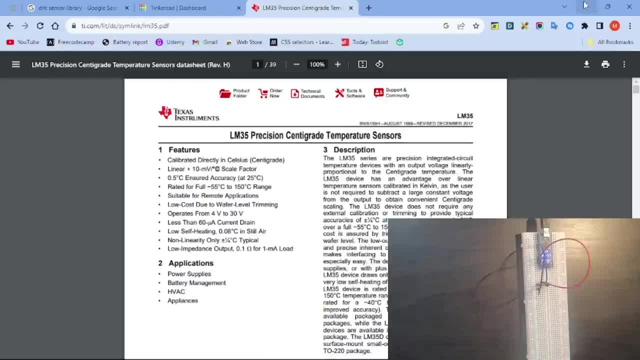 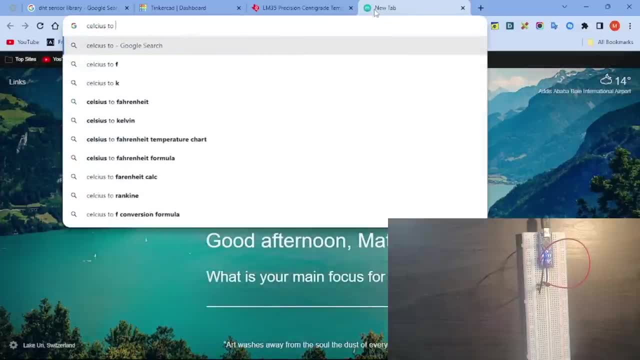 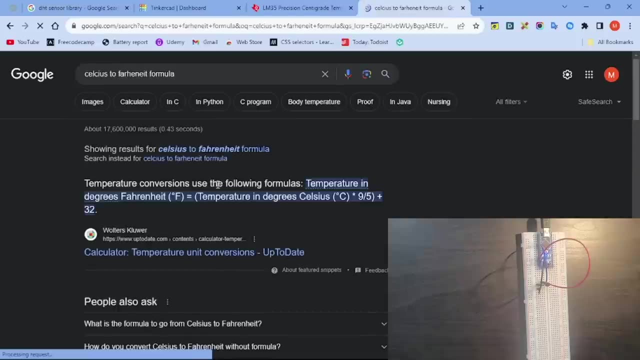 because i think it's simple. but if you have not done it, we need to do this. first, paint formula: what is the formula of? what temperature celsius to fahrenheit, fahrenheit formula. just find that formula right here. all right, there we go. temperature degrees: Fahrenheit is what? 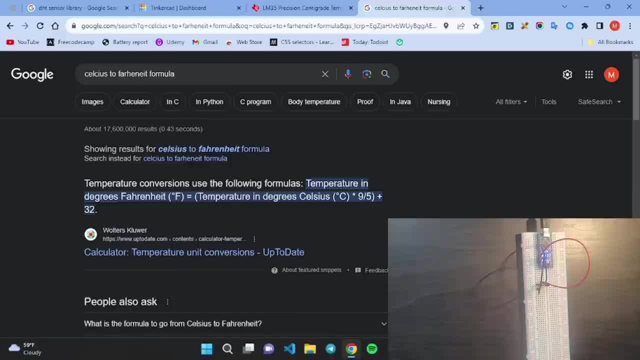 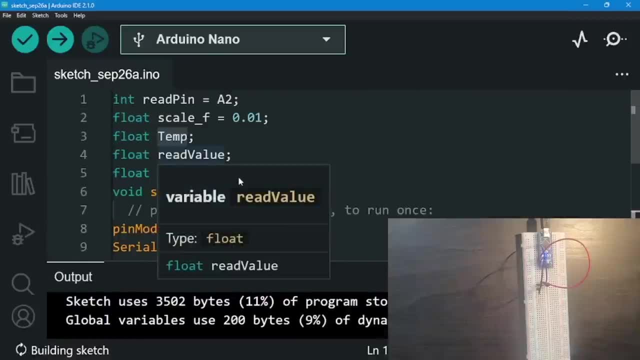 temperature and degree. celsius times nine over five. let me just go over. and first what: assign a variable for fahrenheit? all right, let me just do that. let's go right here and let's say: you know what float float, what float temperature? let me just put capital f just to say it's fahrenheit. okay. 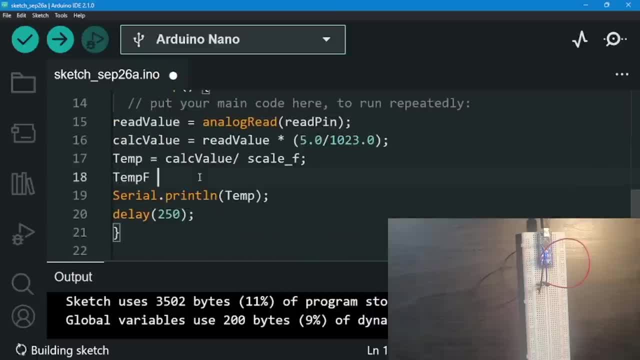 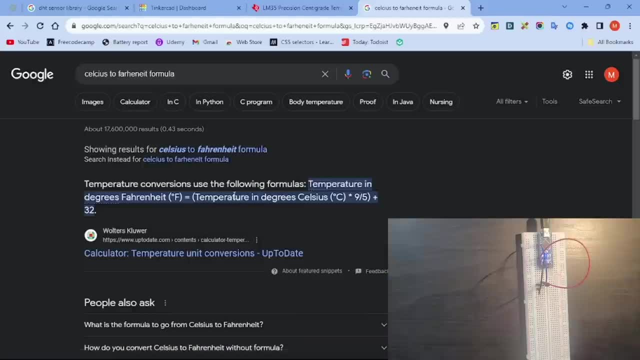 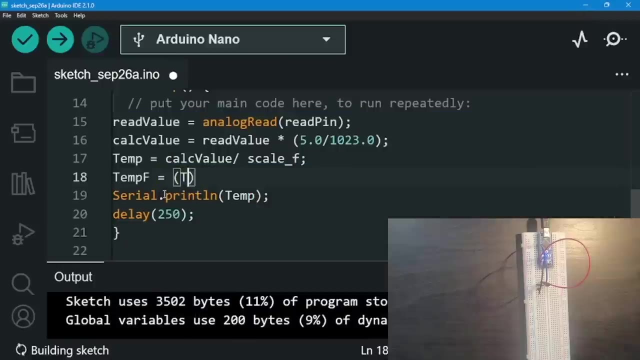 so let me go right here and say: temp f is basically what. what did it just say? let me just go back to my chrome and try to read the formula right here. it's what temperature and degrees celsius times 9 over 5.. okay, that's simple. temperature and degree celsius is given by temp. right here, then we're going to. 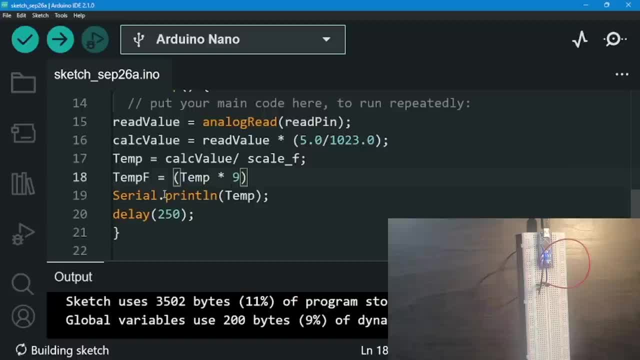 multiply by what, by 9.. again, we need to put what, because we're dividing. what do we need to do? we always need to use a point, 9.0, or we get 9 point. again, it's up to you, 9 point and put a dot. 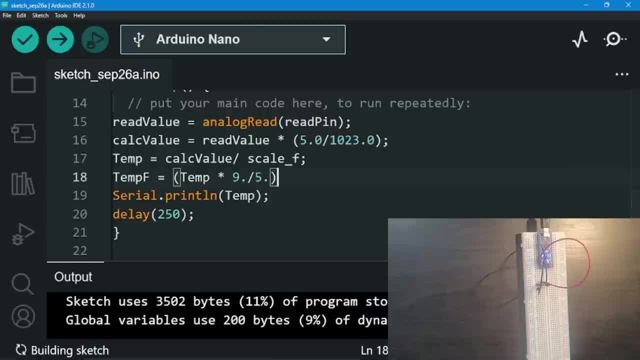 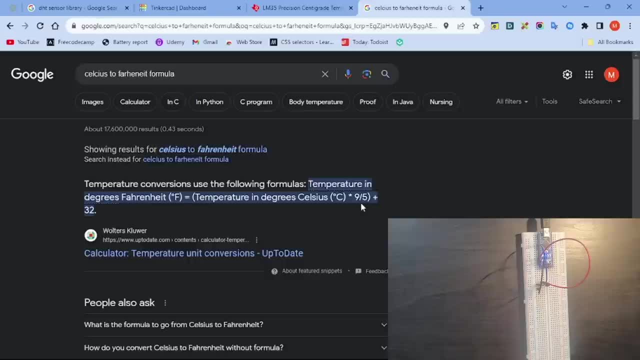 at the very end, dot. there we go. what else do we need to do? let's check that out. and then we're going to add it up by what? by 32.. okay, we need to add it up by 32.. okay, and then add it up by 32.. so one thing that is confusing. 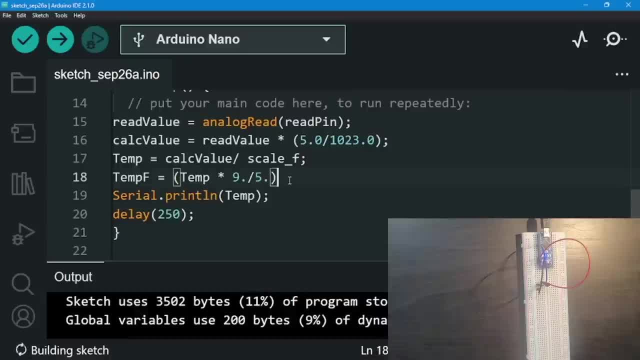 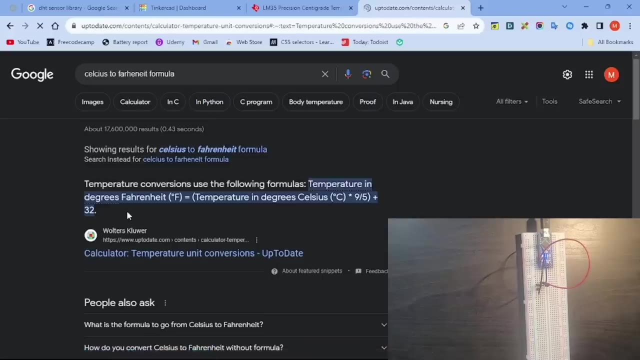 a bit for me is: uh, am i supposed to multiply both of them by 32.. i'm sorry, am i supposed to uh, multiply the whole thing by 9 over 5, or am i supposed to just multiply temperature by 9 over 5 and then add 32.. uh, so to just check that, let me just go right here. actually should be giving to. 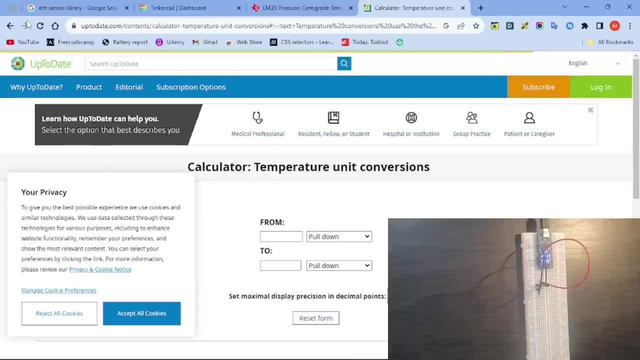 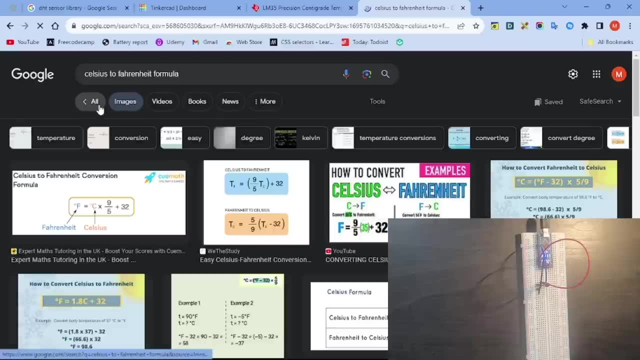 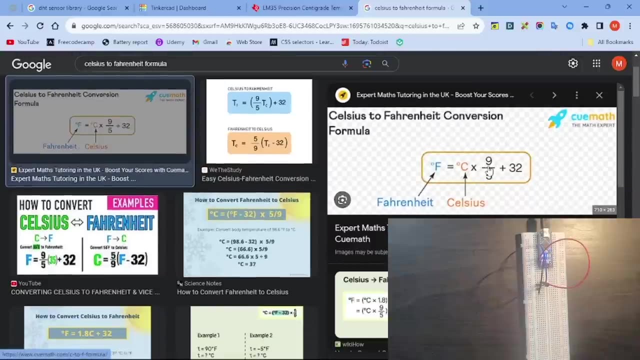 giving it to me on. uh, actually wait, let me just go to something that was written by him, so let me go to images. all right, there we go. now i can clearly see the temperature has to be multiplied by 9 over 5. not the whole thing. you see that. it's not the whole thing. that's going to be multiplied by what? by? 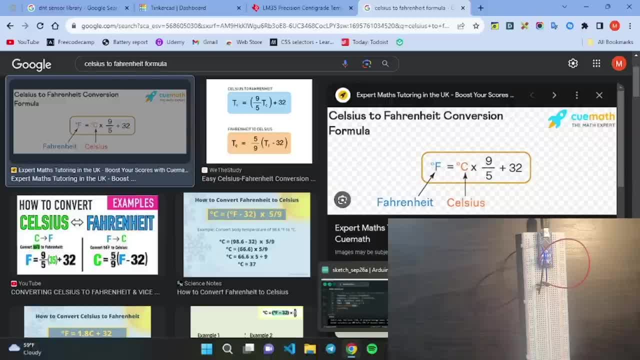 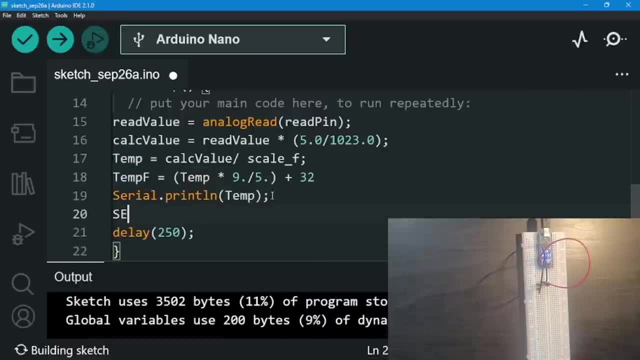 9 over 5.. only the celsius will be multiplied by what? by 9 over 5.. all right, i just wanted to get that up on my mind, right there off my mind. so what i wanted to do right here is serial and get printed. 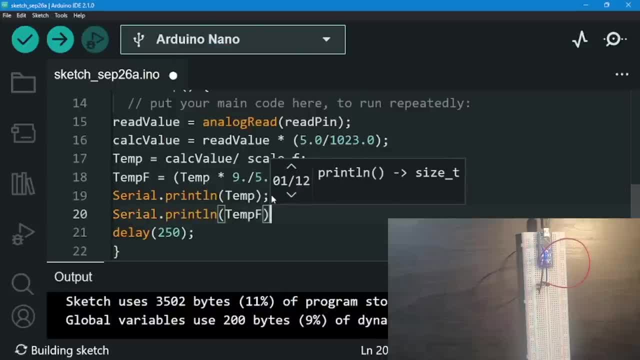 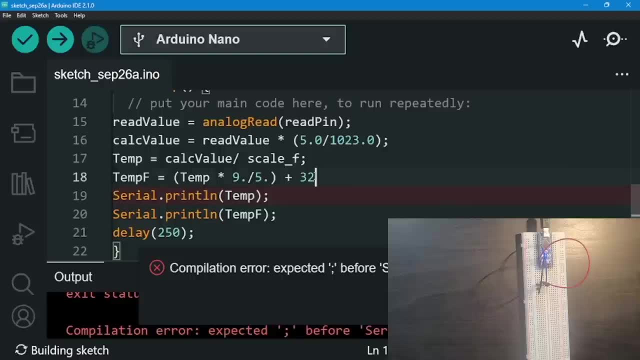 new line temperature f. okay, seems good. now let's try to upload it. oh, i forgot to do what: put a semicolon at the very end. i should have done that right. let's just upload it right. now should be working. it's done compiling and i think it should be uploading. all right, there we go. let's go back. 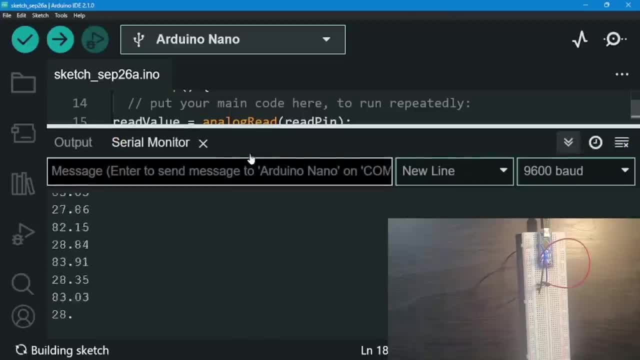 to our serial monitor right here. let me just extend it. oh, we're receiving lots of values, but obviously it's getting a bit confusing here. we do not know which one is the degree celsius, and we do. we do not know which one is what, which one is the degree fahrenheit. so what we're going to? 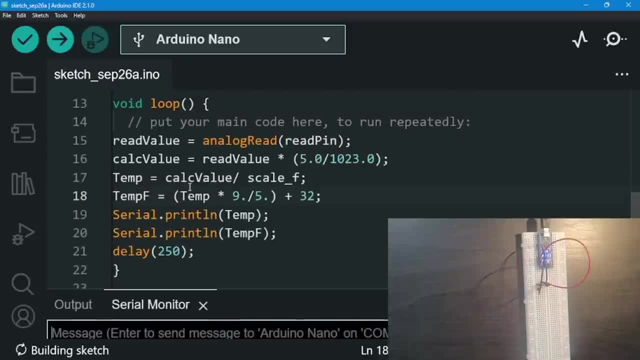 do right here is you know what for degree celsius? let me find degree celsius right here. it's just temp celsius. what i want to do is before this: what i want to do is basically serial dot print, okay, next to it a string: celsius, literally celsius. 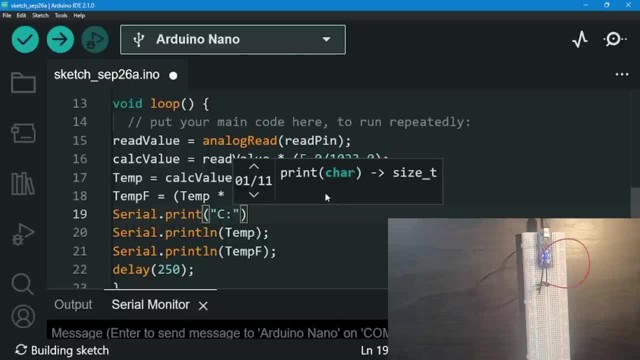 basically what celsius? let me just say celsius c as an indicating celsius, and i'm going to need space. okay, let's say c for specials. and i need to do is what serial dot print for what? for fahrenheit? one thing that is important here to notice is what it's not print. 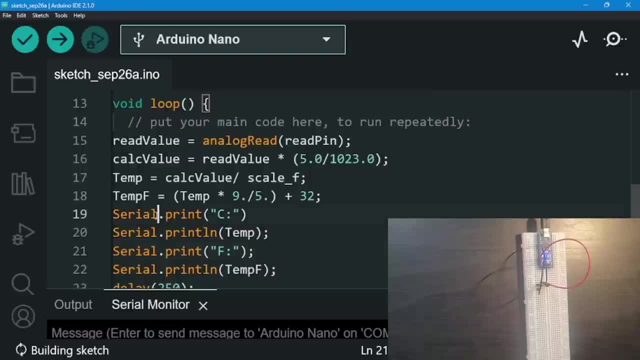 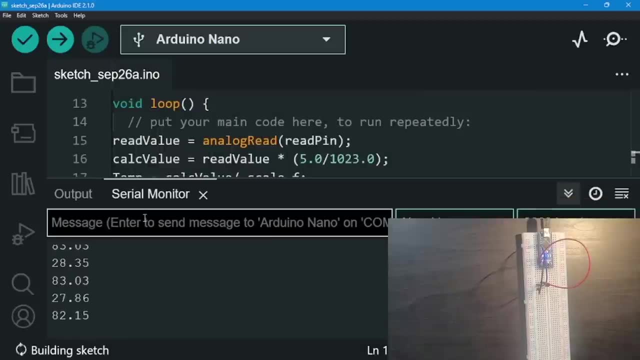 ln, it's print. so, basically, what happens when you print? by the way, what happens when you print something in the serial monitor? what happens? let me just go over to here, my screen. let's say i'm printing 25, all right, 25 is, let's say, the degree celsius. let's not forget to focus on the, on the. 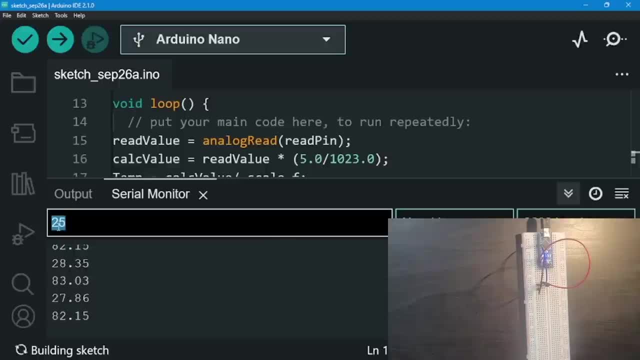 value of the serial monitors books here on the writing. okay, so 25. let's just see that. what's going to happen here. well, basically going to happen is what, first c is going to be printed out- okay, c, and then what it's going to be print what, what is going to be printed next to it? 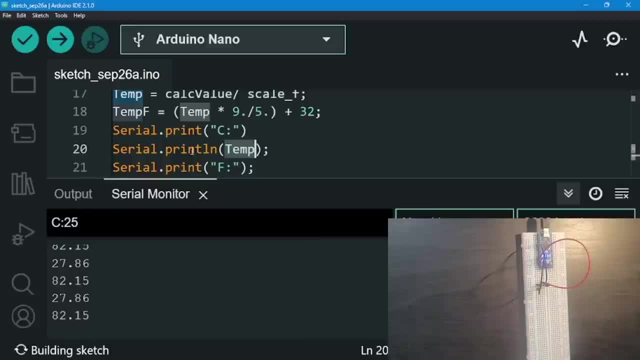 temperature is going to be printed next to it. basically, let's say, it's 25, right here, it's going to be printed next to it. that's what i expect again. so so i'm going to expect this and i'm go. what do i expect next? so let's see, actually, if my code is. 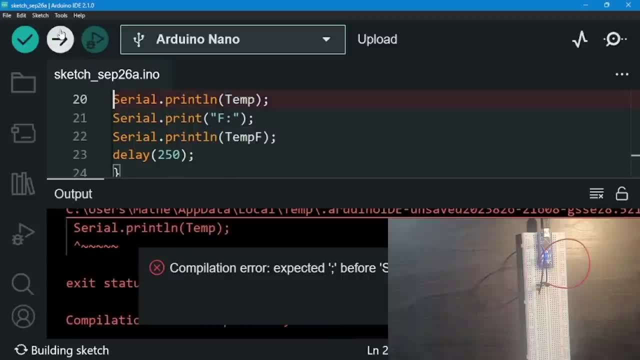 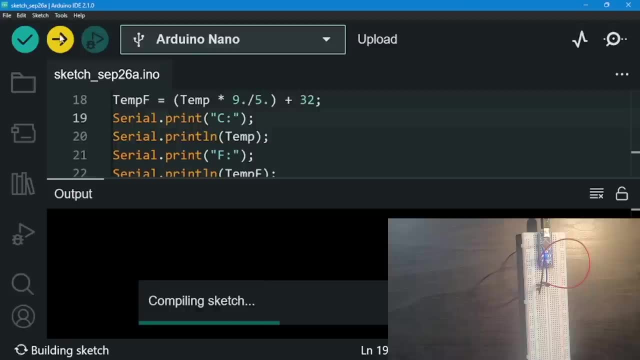 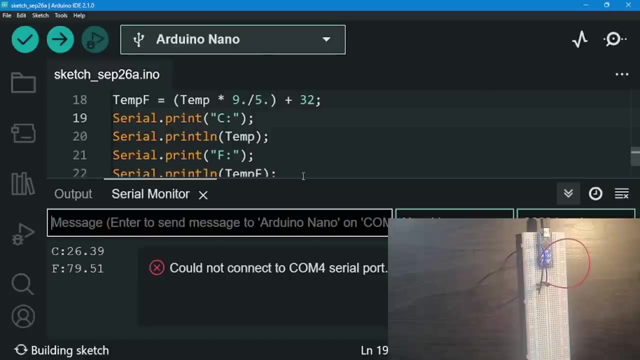 even correct, because i've never used this before, so let's see if it. even if it's correct- uh, i keep forgetting those semicolons at the very end. it's my bad, then i'm just brushing it a bit because i have to go back to the dht sensors. all right, come for it. all right, there we go. 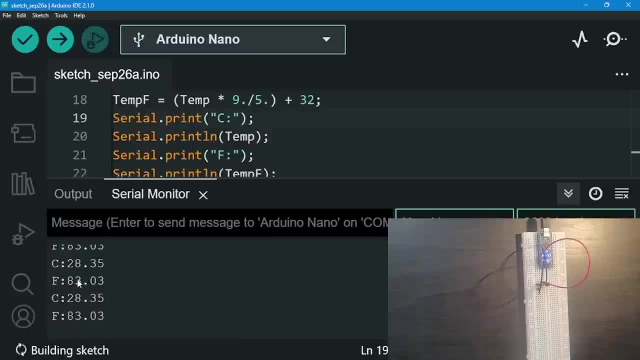 you see that we're receiving: c is 27, fahrenheit is 83.. we're receiving data very fast. speed- you guys can see the fluctuates a bit, but much of the last is the same. so let's say, right now i'm just going to read one of it, let me just take off this toggle. 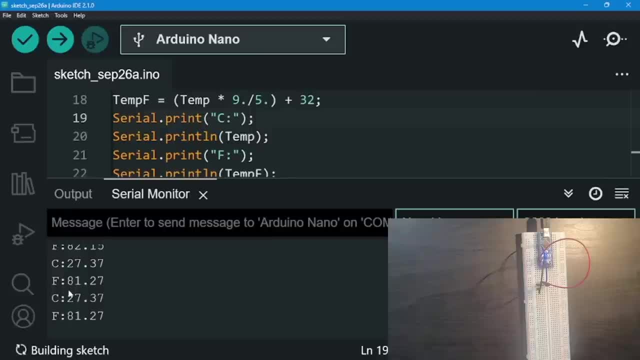 okay, the automatic toggle. let me try to read this one saying: what 27.37 degrees celsius, which is basically what 81.27 degree, what fahrenheit? so again, i have another homework for you and this is again predictable. but i have a simple homework for you, which is going to be that i want you to convert. 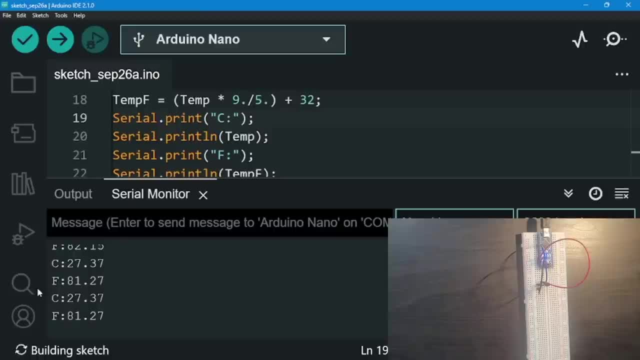 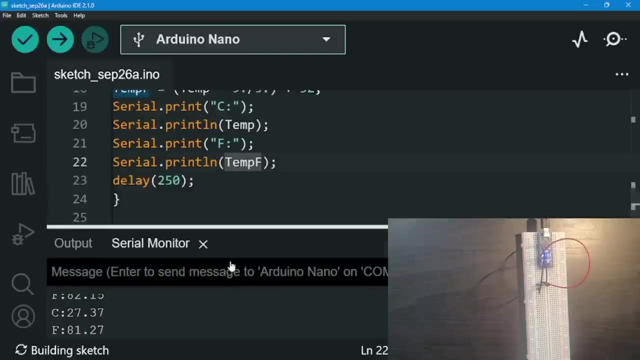 it to what to degree kelvin, and i want you to output what fahrenheit celsius kelvin. i want you to output fahrenheit celsius kelvin. so pause the video and do that. okay, so i suppose that you didn't yourself, but if you've not and you want to be, you know, you want to make sure that you did it right. 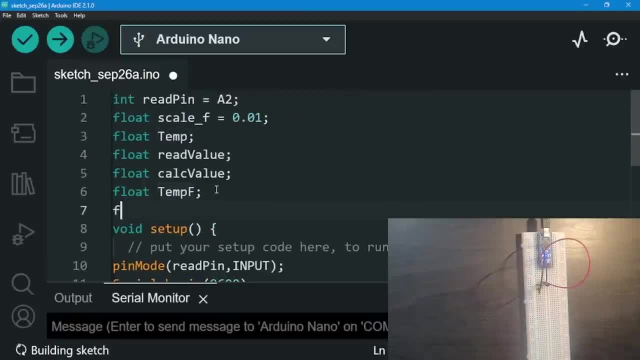 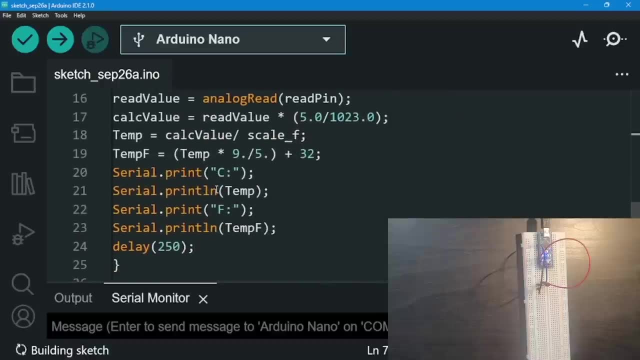 let me just go right here. well, basically, uh, temperature fahrenheit is, it's basically temp k, let's write that down. but basically, temperature kelvin is just adding 270 degrees at temperature celsius. that's all you need to do. so let me just define it right here. 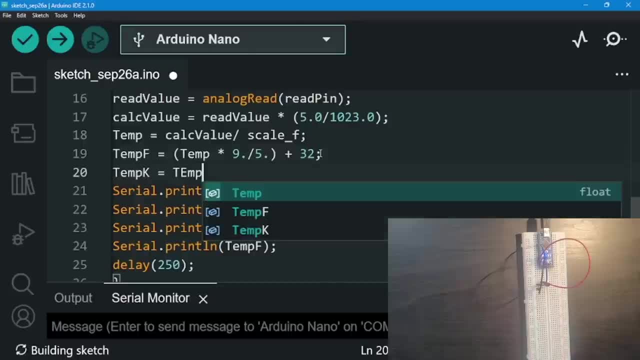 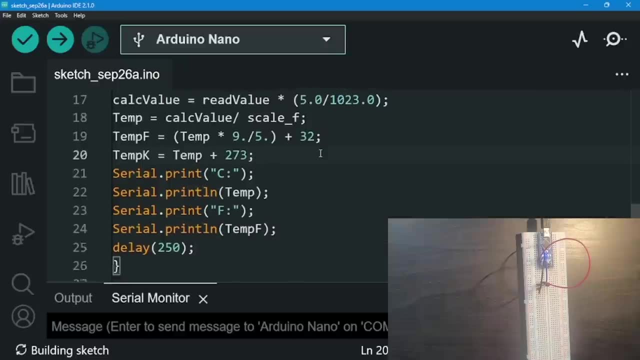 temp k is going to be what? it's literally adding 270. it's going to be like 10 plus 270. that's all you need to do. all right, that's all you need to do. so all you need to do right here is again: we want. 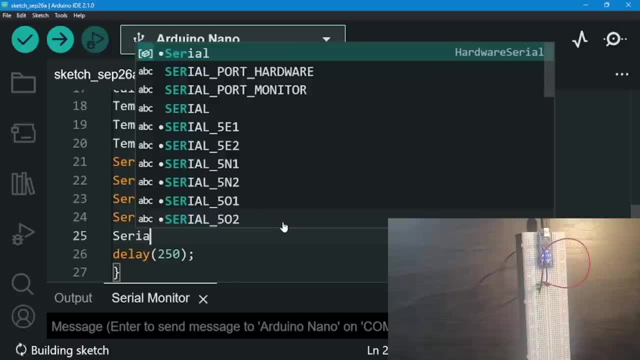 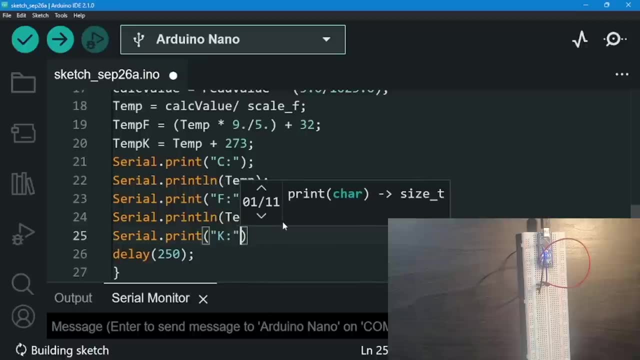 to print it. so we're going to say serial dot print, not ln, only print. we're going to say k again, put a column right here, finish it with a semicolon. let's say: serial dot print ln, new line. and then we're going to print what? temp k, capital k. let me just finish this with a semicolon right there. 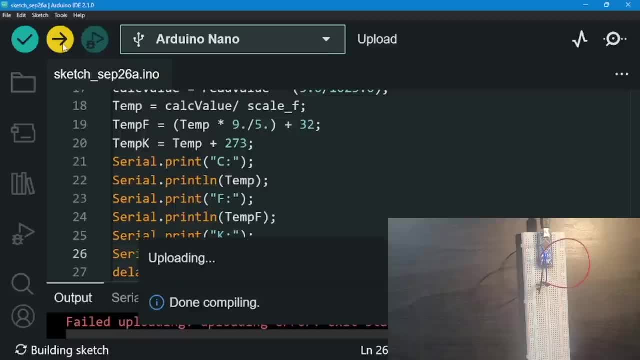 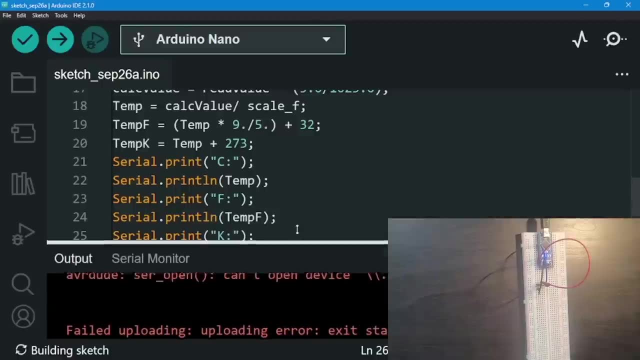 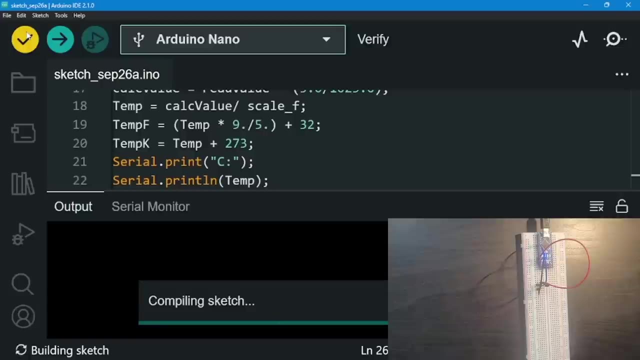 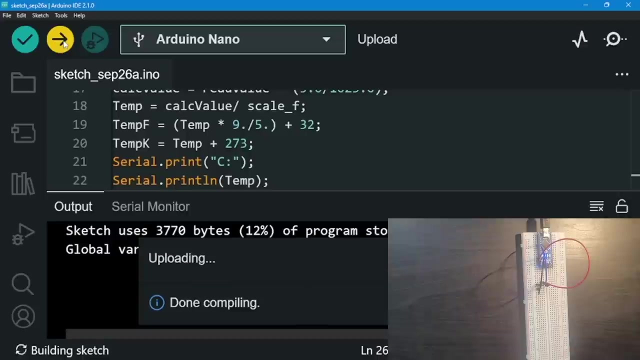 okay, and let's upload it. okay. it's saying: there's an uploader, i don't know why. let me check it again. can't open device. let me just try to run it again. let me just compile it. okay, the compiling. there's no problem in compiling, so let me try to upload it. so there's most likely a problem uploading. hopefully it's not. 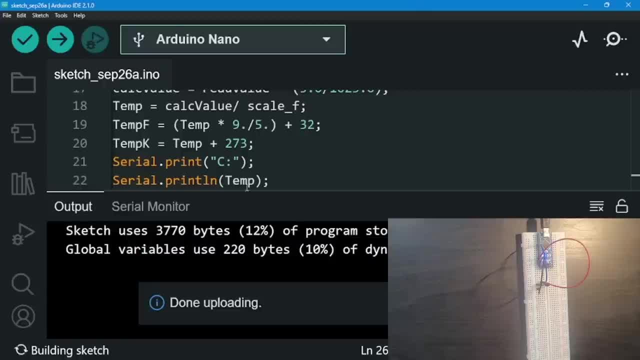 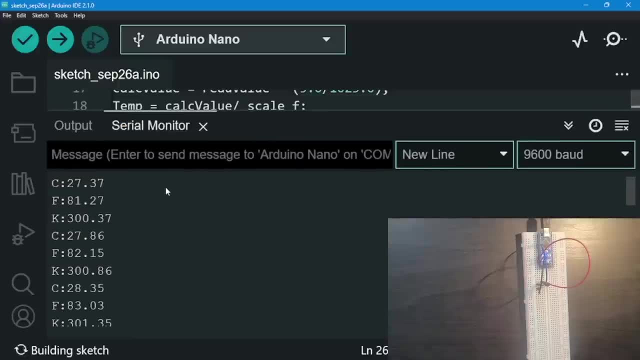 going to happen yet. okay, it's still uploading, all right. all right, there we go. let me just clear this up and it should be running. there we go. you can see c is what f and then a k. we see a c and an fk. f and a k, c and an f and a k. that looks beautiful. let me just go to the bottom again. i just wanted. 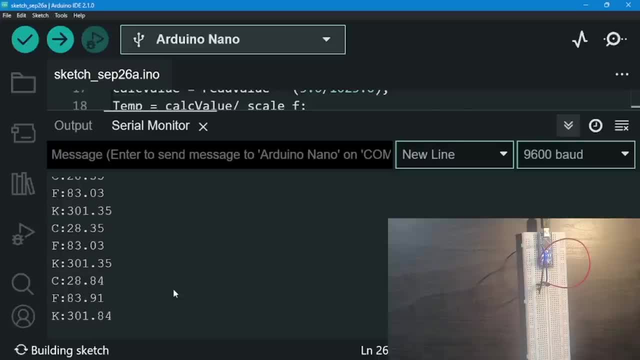 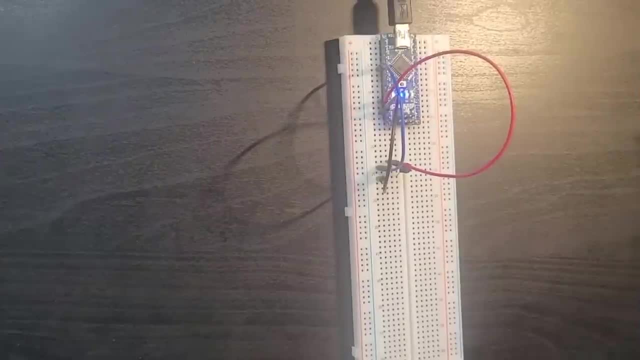 to toggle to the bottom and if itself. but you can see it. yeah, what c, f and k coming simultaneously? all right, that's all you need to do. when it comes to words temperature sensor. i wish that i could bring something colder and hotter right here so we can see the temperature move around. 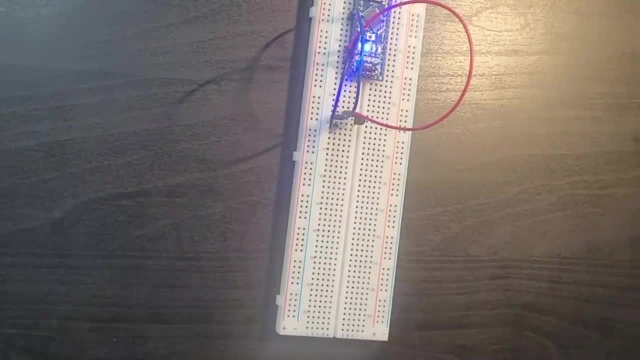 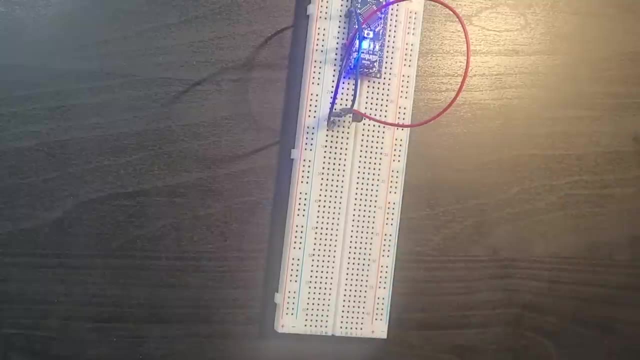 but mostly when it comes to temperature, it doesn't change a lot, okay, and again, i don't want to bring something that's very hot. that's hot, you can plug it in now, okay, so let me just try to do it one more time. or very cold near my arduino, that's why. but again, you can check it for yourself using a digital. 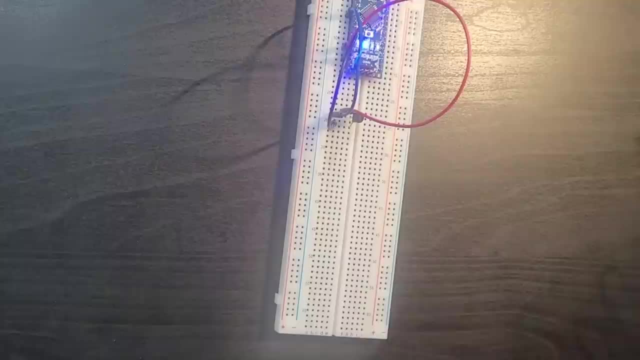 simulator. try to use a digital simulator and again try to toggle around, mess around with these temperature sensors. it's up to you. okay, you can do that or use again. be careful when you're doing whatever you're doing. so, if you're using something hot or cold, be careful when you're putting it. 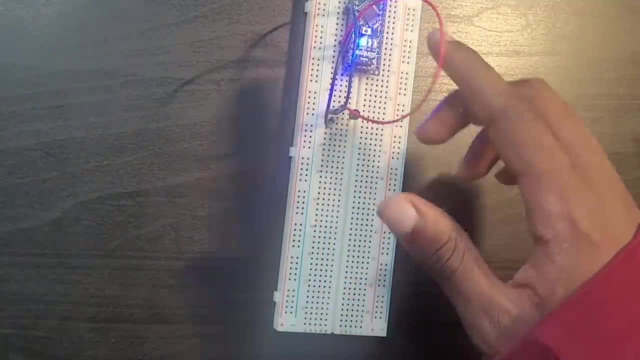 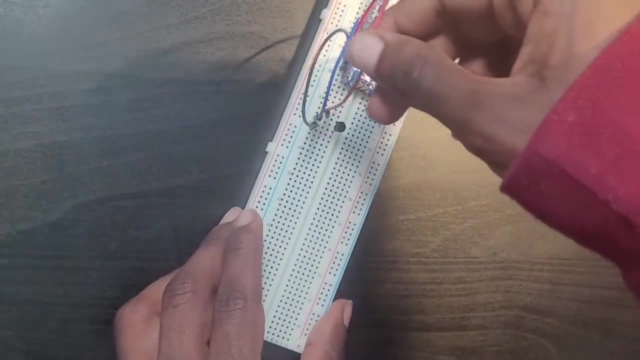 close to the, to the, to the sensor, okay, be close, especially with the wires, okay, because they can really just block your view right here. so you need to be close again. you need to be what, you need to be cautious of what you're doing. so if you're even thinking, thinking of bringing something, 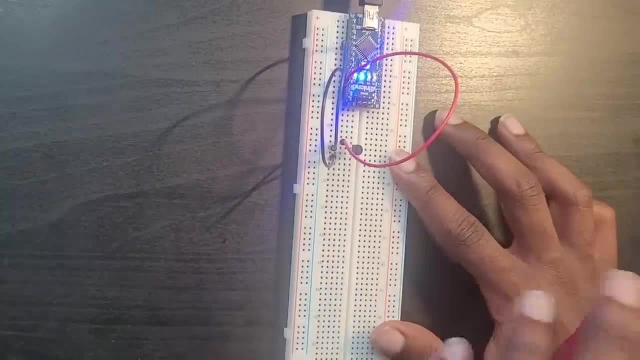 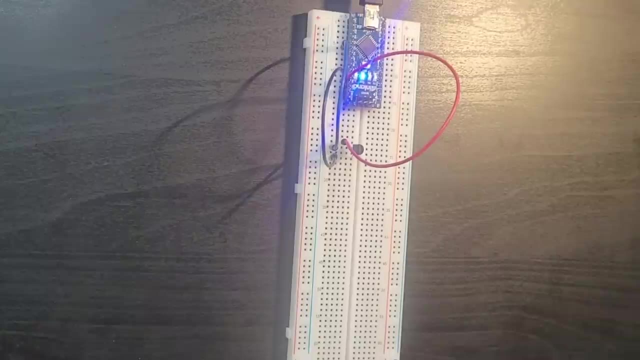 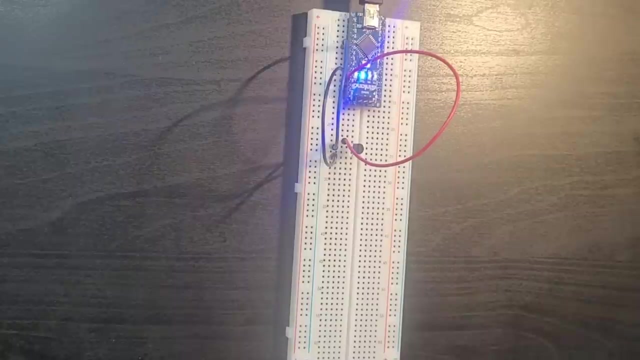 cold or hot, to just again check the temperature sensor. be careful about it. okay, so that's about it for the LM35 sensor and for those of you have again DHT, we're actually going to see the DHT sensor. so you guys, I might as well skip the DHT sensor because I don't think you're going to be using. 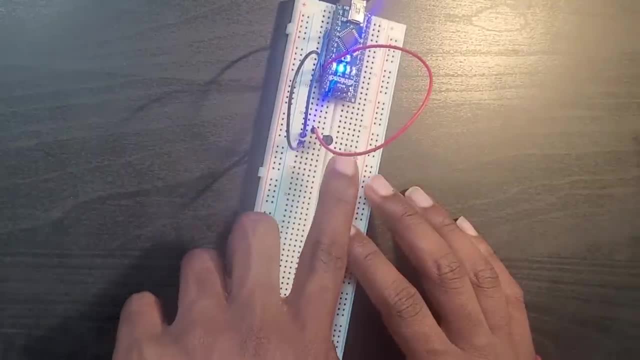 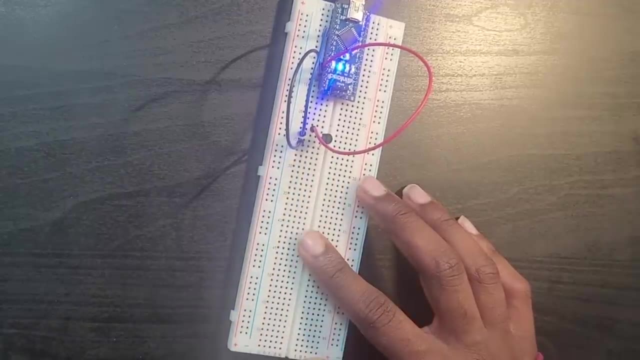 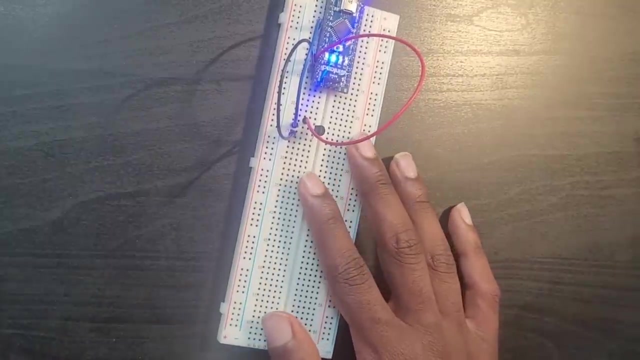 it if you have an LM35, okay. so for those of you again who wish to, who watch this section, are going to be using the LM series: the LM35, the LM36 and all these series, okay, the ones that use the LM. obviously, what I want you to do is what I want you: to skip the next section, because I'm 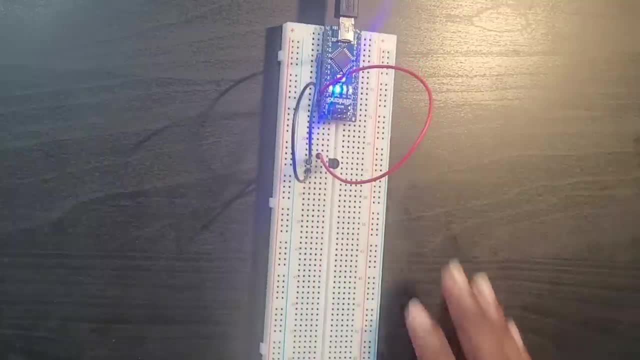 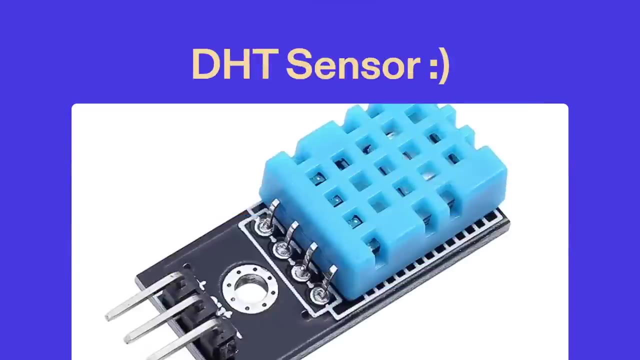 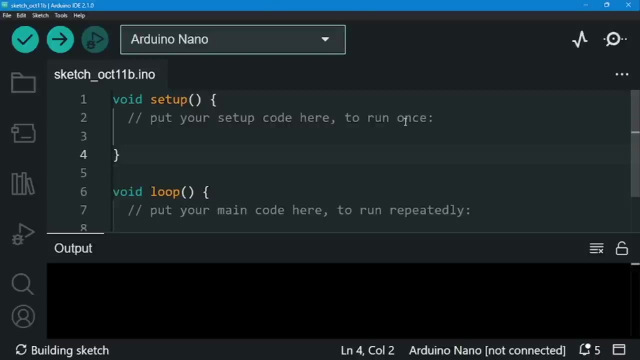 going to be talking about DHT sensors, okay, so keep that in mind. so see you in the very next section, okay, so now let's talk about the DHT sensors. okay, so one thing I want you guys to keep in mind when it comes to these temperature sensors is: there's a lot of them. there's the DHT, there's. 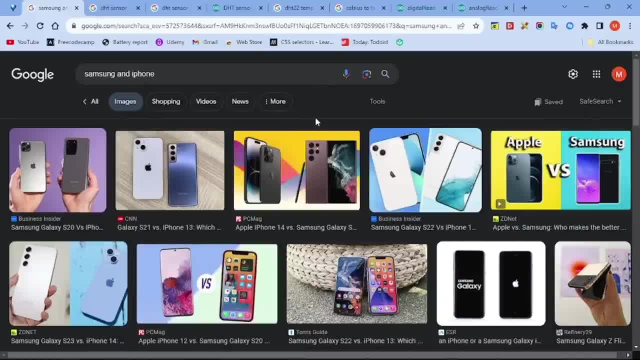 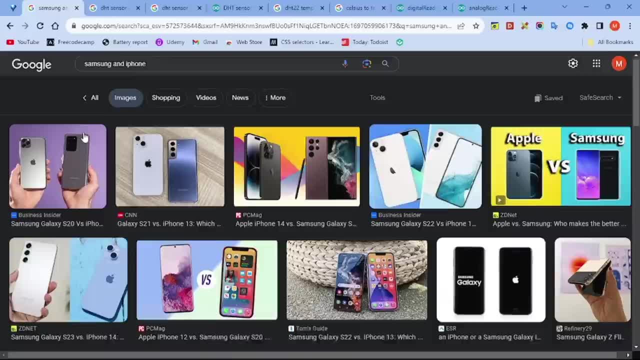 the LM35. there are even different types of- again, sensors that are, again, unknown. okay, so one thing I want you guys to think about is what I want you to think of them as Samsung and iPhone. so when you look at them, both of them are phones. they have a lot in common, but they also 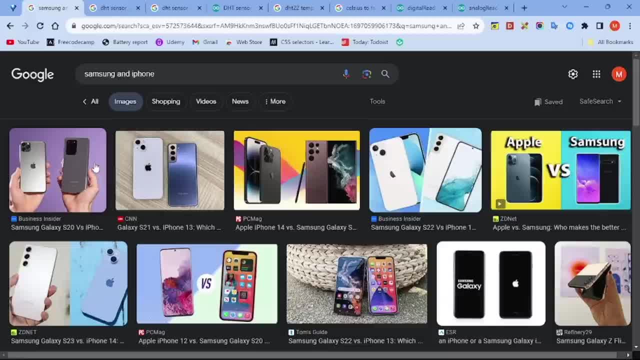 have their differences, so obviously they look different again. they have different features, but they do what? basically the same thing. so they what they make us. you know, we can use it to what to call. for example, we can take photos with it, we can use apps with it, okay, so one thing I want you guys to 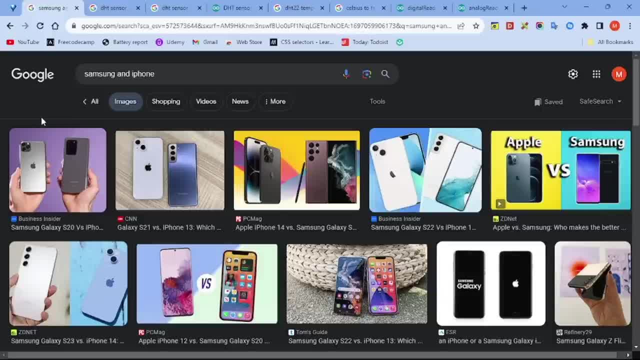 keep in mind when it comes to temperature sensors is there's a lot of them with different numbers, but they have what? that they are mostly the same. all right, so they have again difference in features, and again difference, and again how they look at all and how they're hooked up again and how they work, but they're what they're. 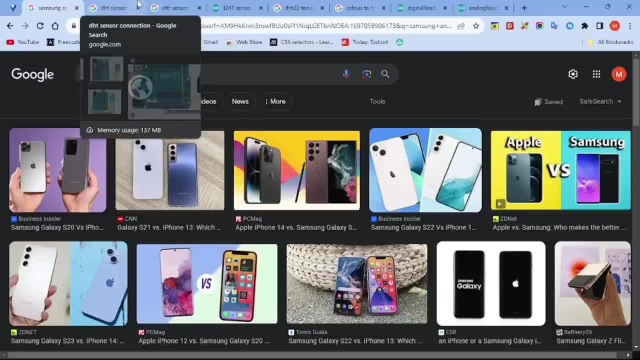 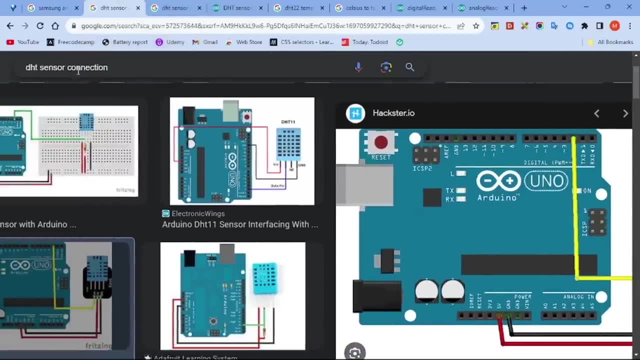 essentially. nevertheless, they're what they're the same, more or less the same. okay, so let's work about the DHT sensors. so you're going to be searching up again your sensors, again the equivalent sensor you have, and check and check for the what, for the connection. okay, right here I'm. 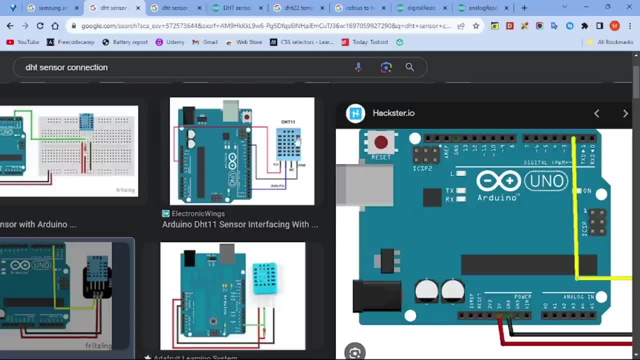 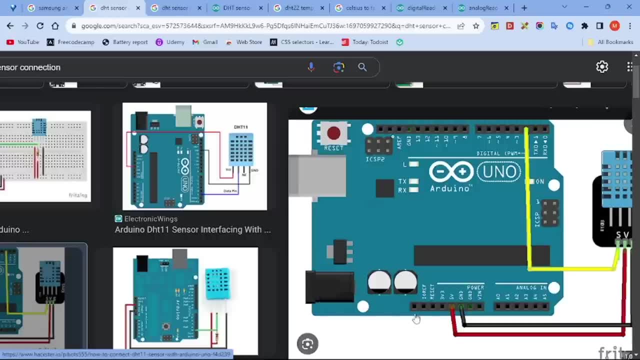 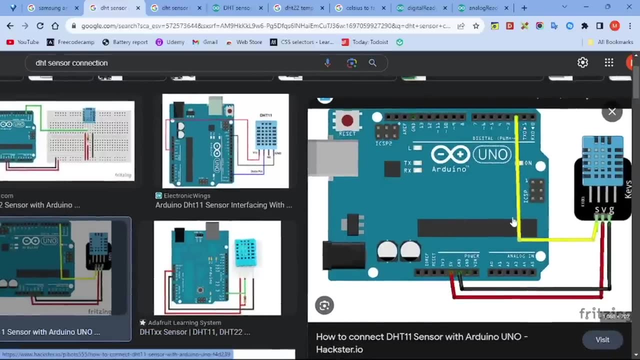 just going to demonstrate using a DHT sensor. so I'm going to go to DHT sensor connection, okay, as one of the most popular pins. so right here, as you can see, just let me just zoom out so you can see the whole thing zoom out. there we go and, as you can see, right here is the most left side is connected. 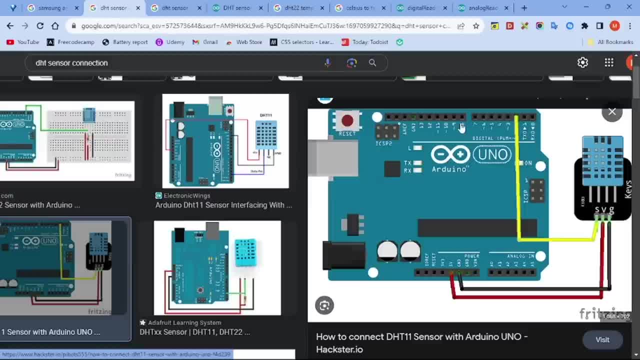 to a digital pin right here so you can use any digital pins right here, okay, and then the middle side is connected to five volt and then the very right side is gonna the GND. so one thing I want you guys to keep in mind is what this thing is going to be using digital read. okay, so it's going. 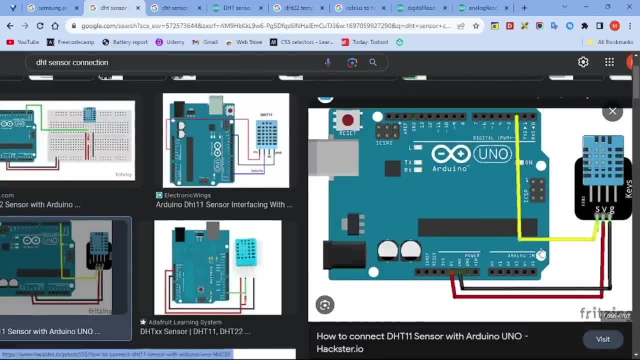 to be digital pins. we're going to be using digital pins, not analog pins for this one. okay, for reading, I think most of you again, we've been using so far what we've been using analog pins to read, okay, from the what from the sensors. but in this case we're going to be using digital pins and I'm going to 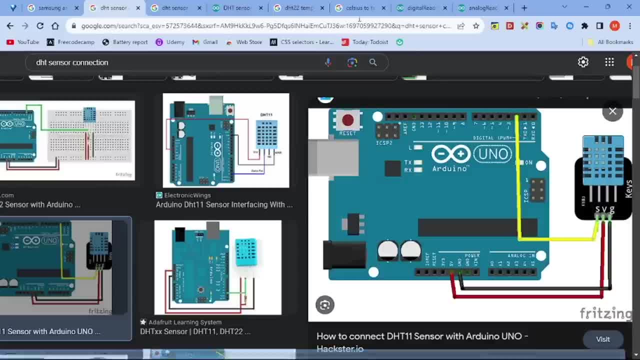 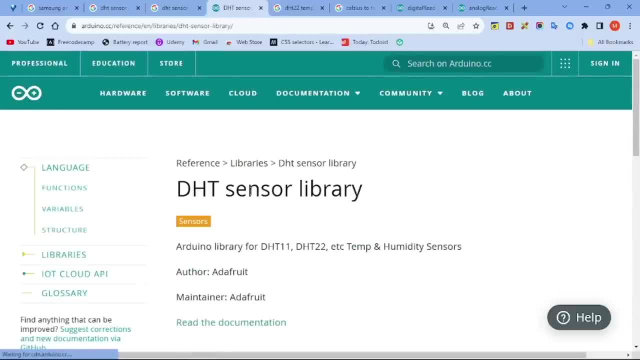 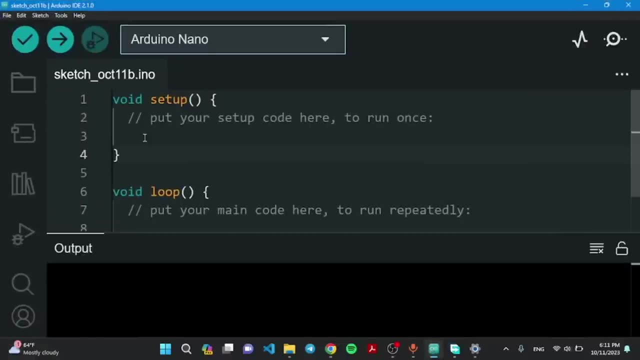 explain um in a bit why. okay, so right here again to make again our lives way easier. we're going to be using a DHT sensor library. okay, so you're going to be using a DHT sensor library. that is by what? by right here. to add, it is: go to Arduino, go right here and go to our again. let me go all right here. 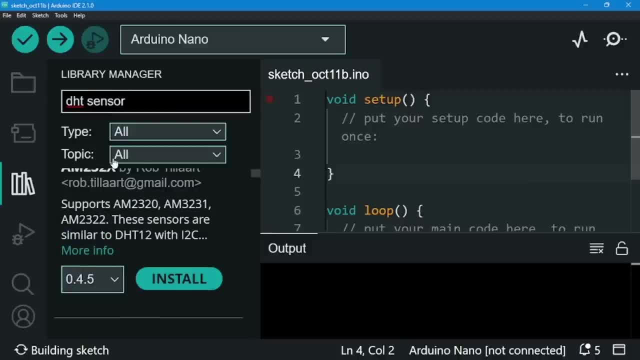 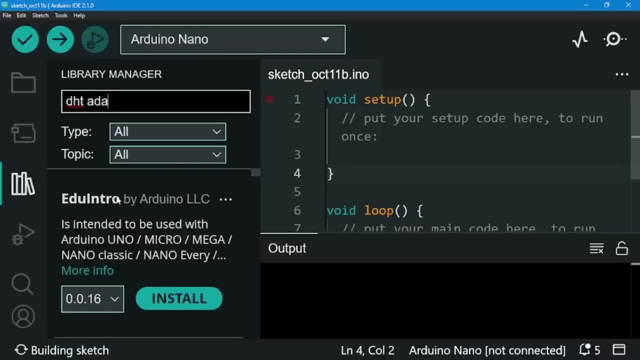 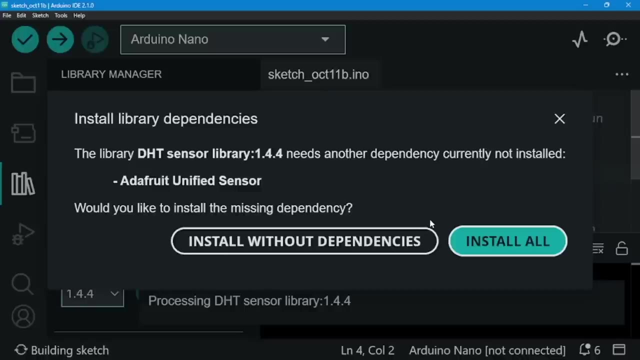 and then search for DHT sensor and try to install the one by eat a fruit. there's a lot of DHT sensor libraries, so let me search for DHT and search for eat a fruit. there we go: DHT sensor library by eat a fruit. all I need to do is install it right here from the library manager and it says that there. 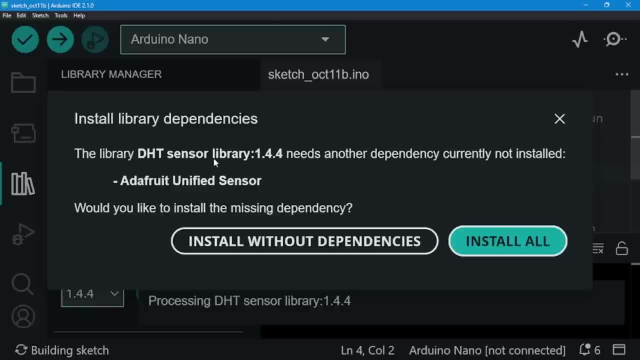 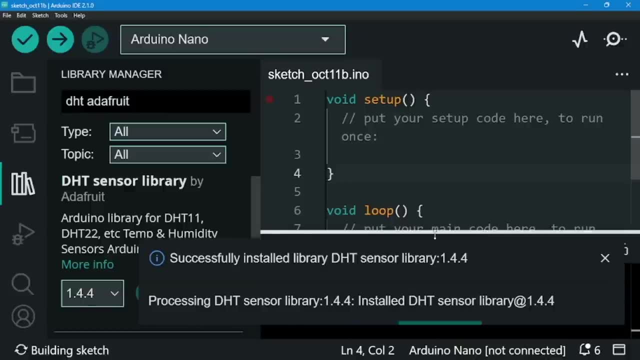 and needs this 80 fruit unified sensor library to be installed. so if it does not, if you don't install this, the code is not going to work. so let me install it all. there we go. let's get both going to install the DHT sensor library and the. eat a fruit- there we go. eat a fruit unified: there we go. 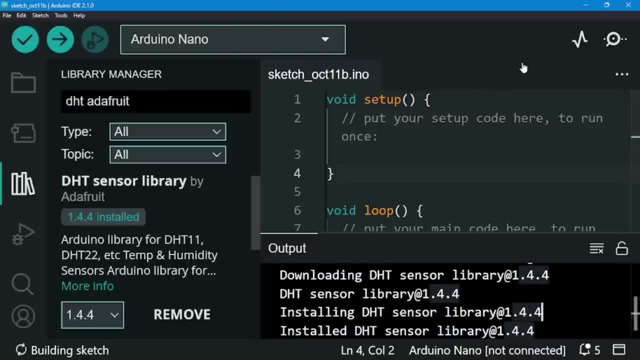 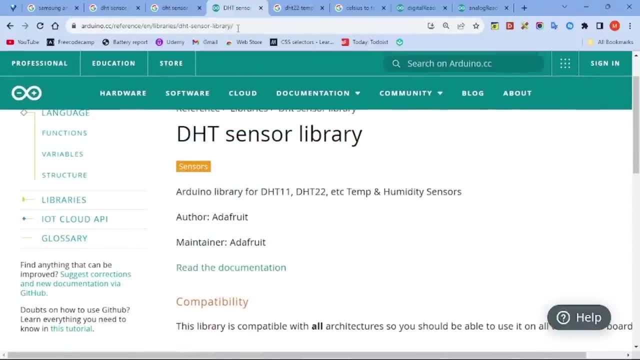 unified sensor installed, both of them okay. so right here, that's what we can do. but another option is again to go to our DHT sensor library again. Google it again by either fruit, and then you're going to find the first link. all you need to do is Google it. 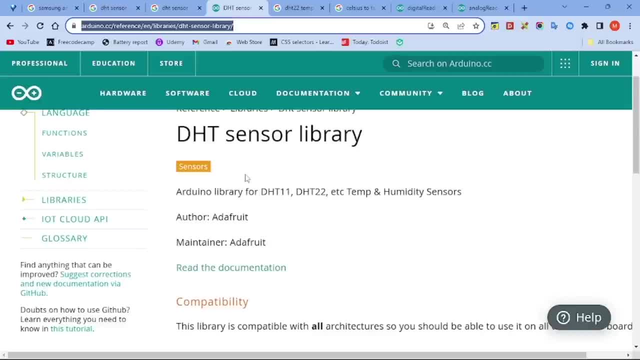 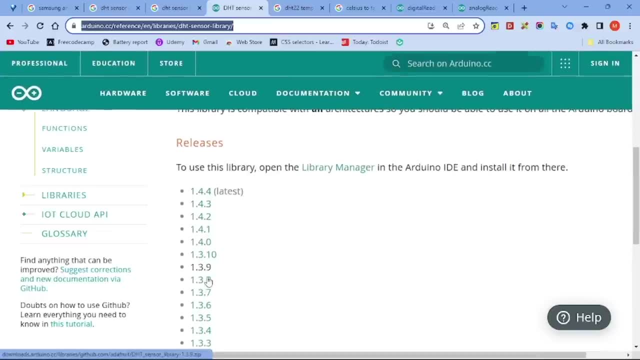 there we go DHT sensor library and search the Arduino link, and then all you need to do is download the version again that you want. so if you don't want the newest version, you can download the Legacy version anyways. once you're done downloading that, all you need to do is add it to go to Arduino. 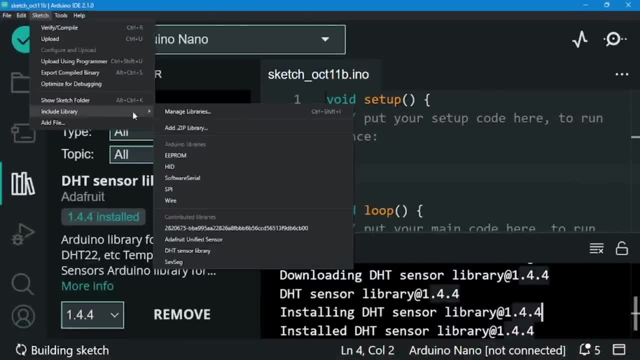 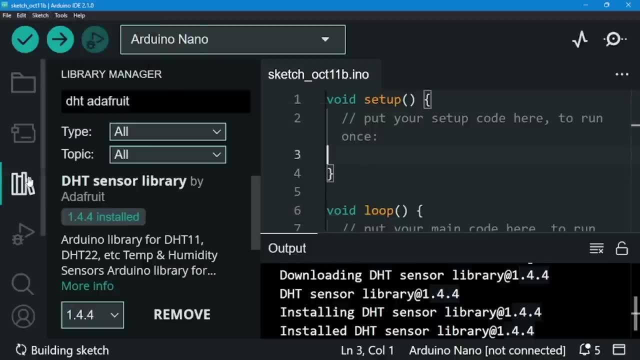 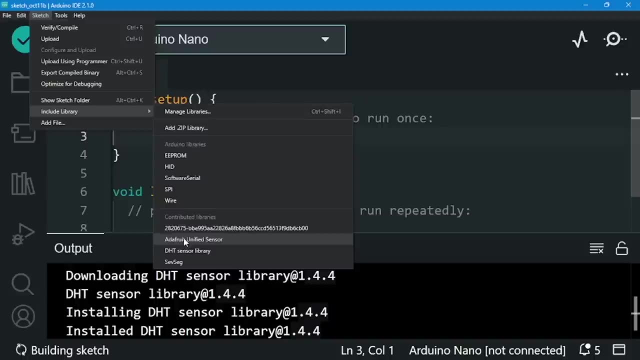 and then go to sketches and go to include library and add it as a zip library, okay, so with that in mind, we're going to be using eat a fruit. so once we're done doing that, we say we go to sketches again and we go to include library and then we go to eat a fruit again. DHT sensor library we're going to be using 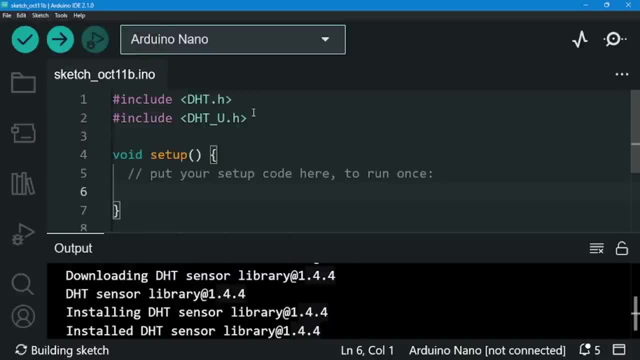 the DHT sensor library. so I'm going to touch that. that's going to include the code for us. so it's going to basically include it and if itself, so we don't even have to write it down ourselves, okay. so again, for those of you want to read the documentation, it's available on the. 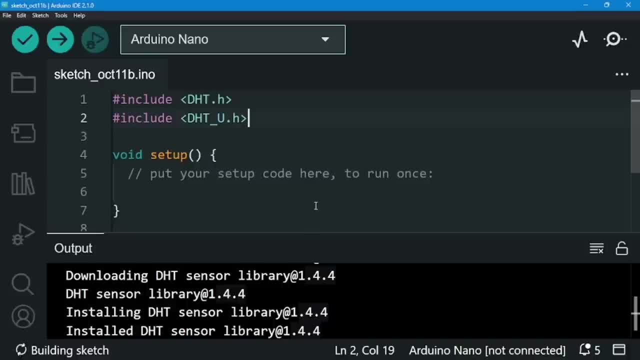 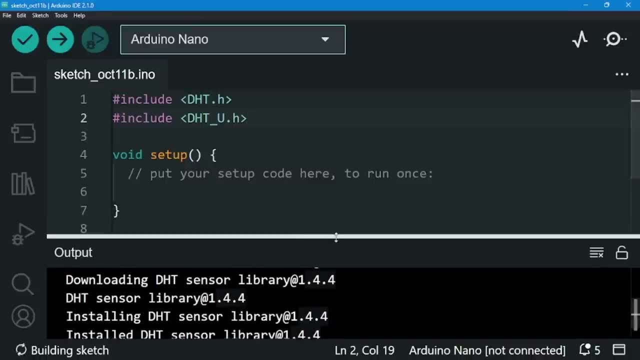 Arduino. so, again, I highly recommend that you guys read the documentation after this video so I can use it for, uh, more things that actually is capable of. so I'm just going to be explaining just basic stuff, okay. so with that in mind, now what we need to do is actually use this, set up this library and 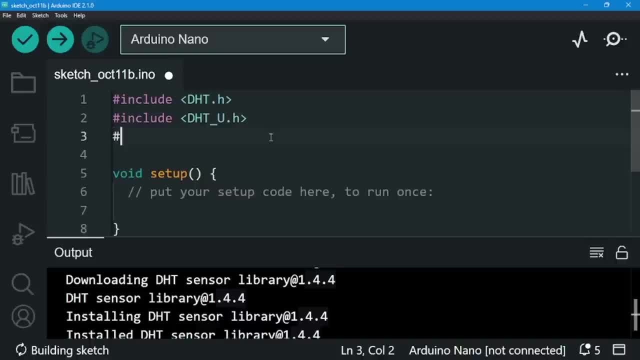 try to use it okay. so right here, we're going to be using define, hashtag, define and then type: okay, DHT, what yesterday? right here at DHT 11.. so you're going to be writing down, type and then writing down the DHT, specific DHT model that you have. so, just like how we have Samsung s20, s21 when it comes. 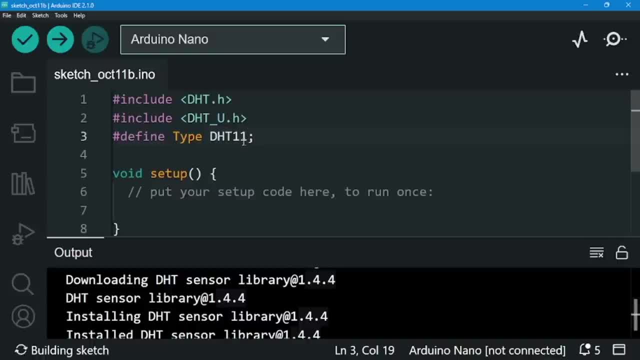 to iPhone 11, iPhone 12 and all of that. we're going to be writing down specific model of the DHP, the DHT pin we have right here, okay, so once I'm done doing that, I'm going to be defining what pin we're going to be using for sensing it all right. so, right here, let me look to my connection. let 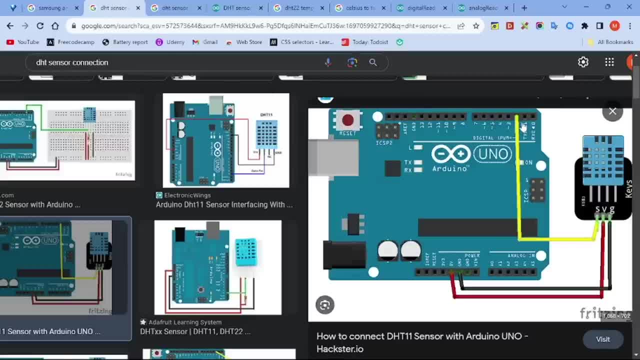 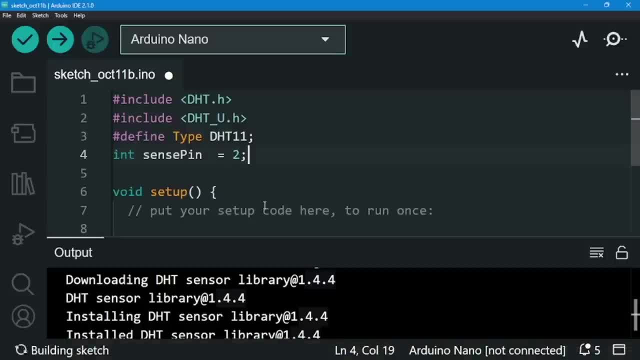 me just search for the connection right here, and it's digital pin two that we're using right here. so let me write down digital print two, so it's going to be equals to what two basically, and then DHT HD, and then we're gonna basically what we're going to give it the sense pin. okay, since pin. 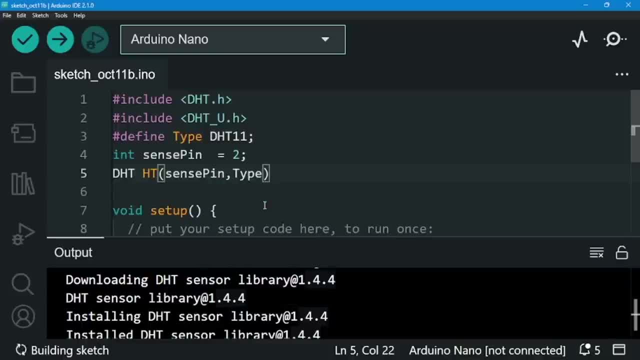 and then it's gonna give, giving it the type of pin that we're going to be using. okay, so we're telling our dhd Library what we're telling it what type of pin we're using and then what we're telling it with the sense pin right here, it's going to be digital pin two that we're going. 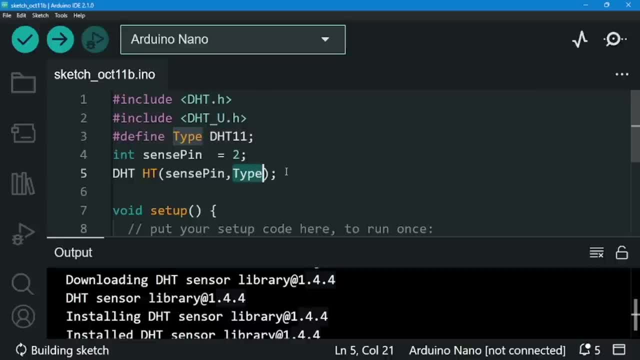 to be using it, and then the type of what, the type of DHT sensor that we have. okay, so, once we're done doing that, one thing the DHT sensor is capable of is it can also sense humidity. so we're going to actually use humidity too, so we're going to be setting up humidity right. 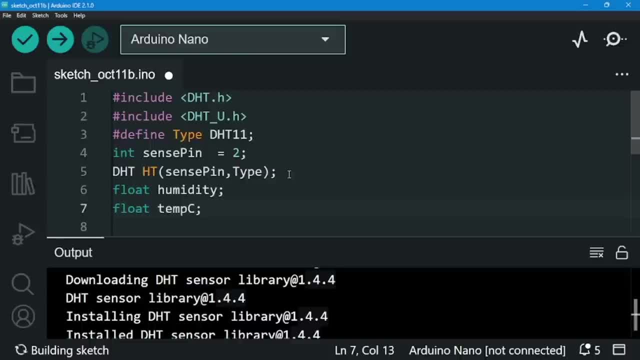 here i'm going to be setting them as again float because they come out in decimals. so when you hear again in degrees celsius, we say 29.6 degrees celsius and everything. so it's going to be again in float. okay, so set it up and float, and then we're going to write down everything we're. 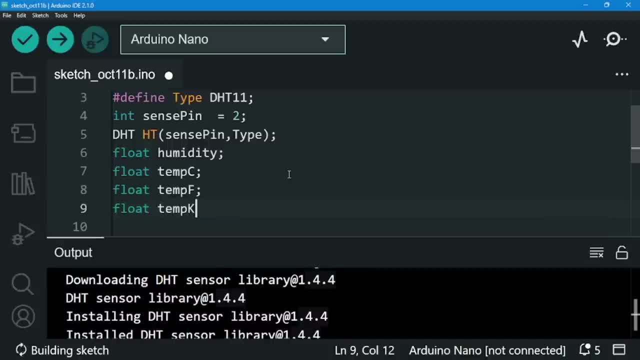 going to be writing them down with the tree, what with the temperature in fahrenheit and kelvin. we're going to be writing them down in three forms, all right, okay, so that's it: humidity, temperature, celsius, fahrenheit and kelvin. once we're done doing that, we're going to need to set up our 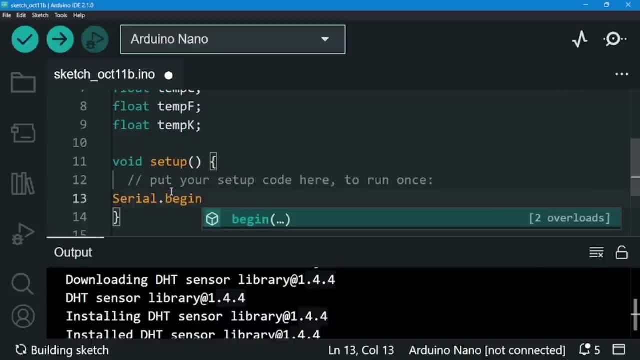 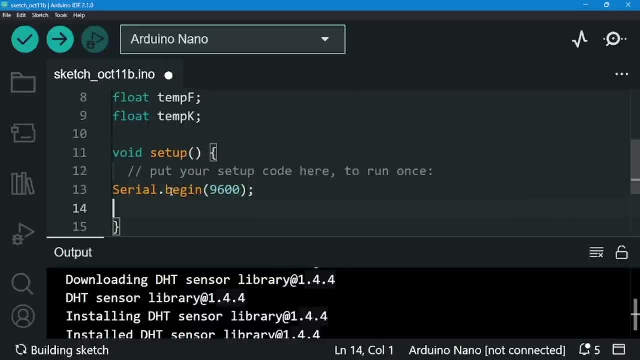 serial monitor, because that's where we're going to be reading our- again our- degrees, okay, so we're going to be reading using our serial monitor, so 9600, as usual, set it up and then we're going to begin. so we're going to be telling what we're going to be telling our dht sensor library to. 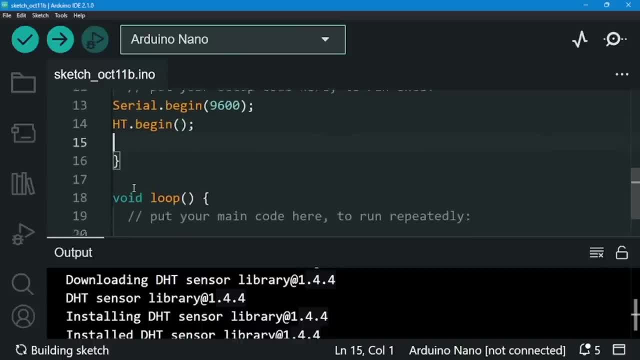 begin, okay. then once we're done doing that, we'll go to our loop code right here, okay, and then we're going to set up again the, the values that we just want that we set right here. so we're going to be again, uh, assigning them the ones that 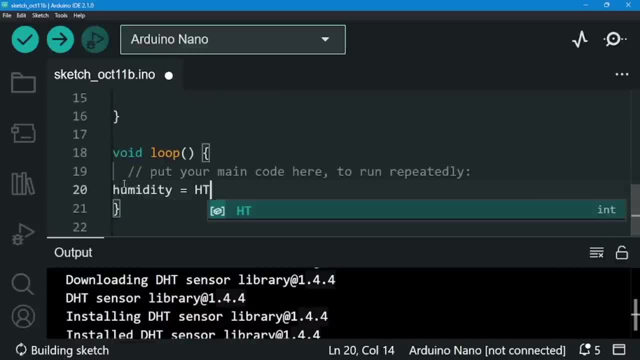 we just set here. so i'm going to humidity and set it to. we're going to say hd, that we already began right here, okay, that we began right here. we're going to be say hd dot, read humidity, okay, read humidity. and we're going to go for temperature celsius and we're going to say hd. to what? 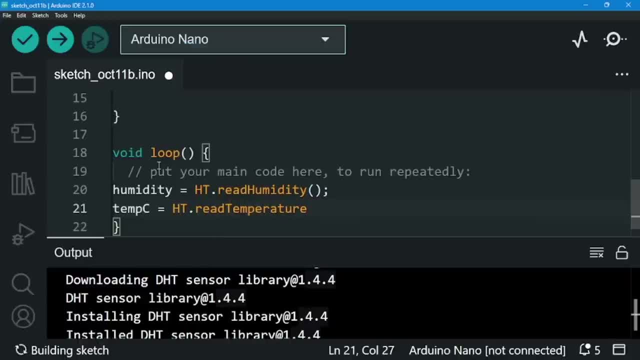 read temperature. okay, read temperature. you can predict this, since read humidity and now it's obviously going to be read temperature. okay, that's what we're going to be basically doing. when it comes to the temperature fahrenheit and kelvin, what do we do? we convert temperature Celsius to. 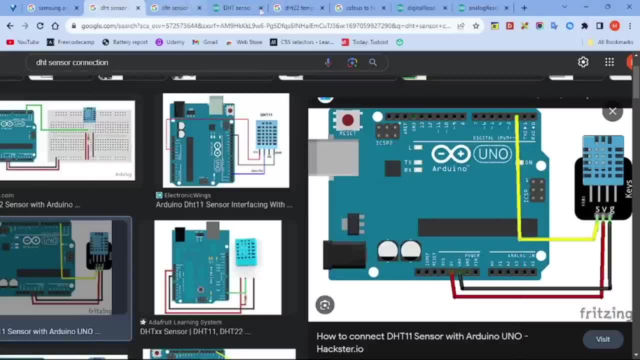 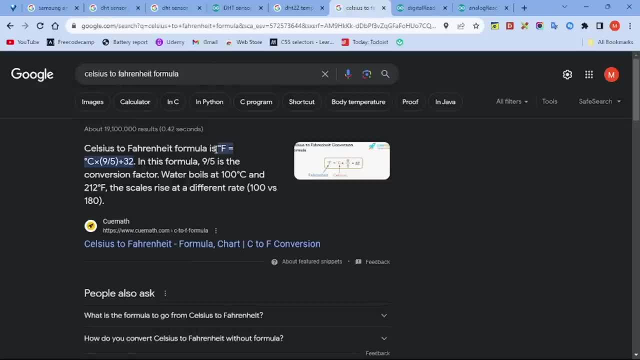 what to Fahrenheit? how do we do that? obviously we use the formula. so let me search for a formula right here: Celsius to Fahrenheit formula. there we go. Celsius Fahrenheit formula- is what Fahrenheit is what degree? Celsius times 9 over 5 plus 32. okay, so I go to my code right here, and then what? 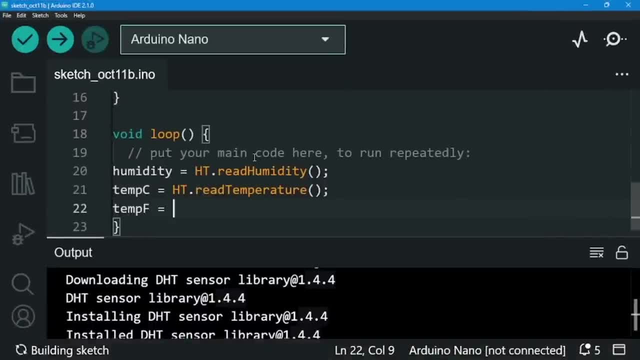 I go to temperature Fahrenheit and say, oh, I want to do is what? I want to use temperature Celsius. I want to multiply it by 9 over 5, plus added with what 32. so right here I did what I did, two mistakes right here, so you guys can actually see it. what is the first mistake right here? 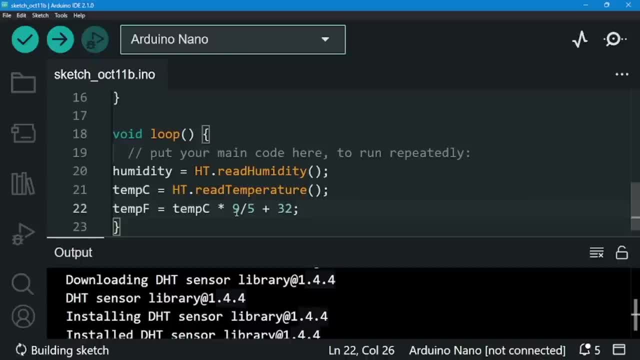 the first mistake is what? we're now using decimals when we're dividing. what do you want to do? we want to use floats, so we need to put what a point or a point, oh okay, that's what we need to do. we do not do that. that's the first mistake that I 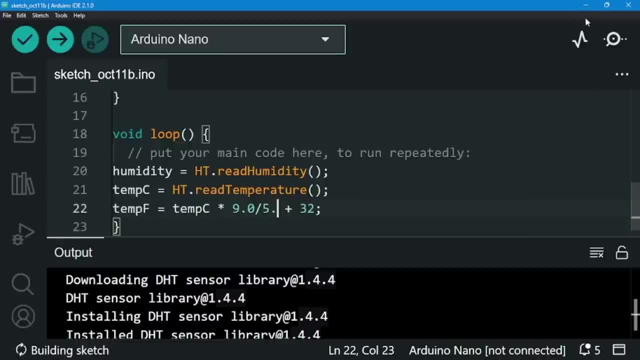 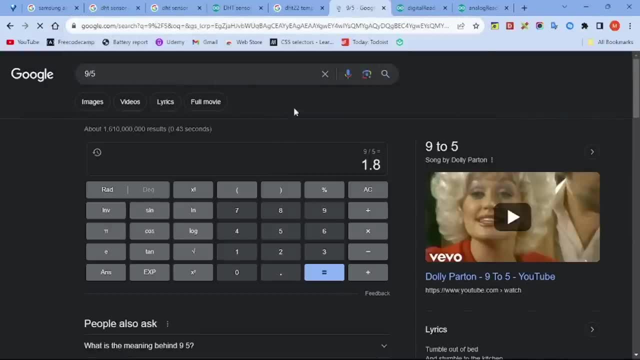 did right here. obviously, if I said 9 over 5, it's going to be what I actually did: 9 over 5 right here. what is the value of 5? it's 1.8 and it's going to round it to what? to an integer right. 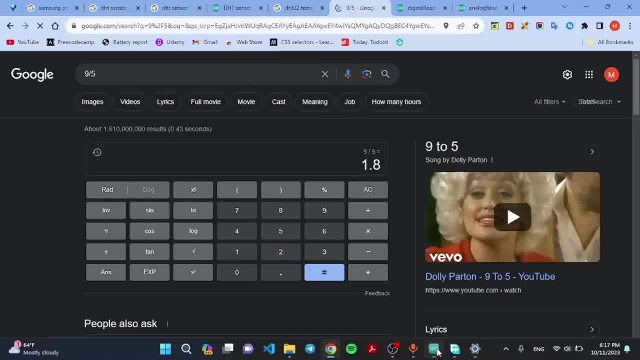 here. it's going to be rounding it to it to an integer. so it's going to be rounding it to an integer. I don't want it to do that. I want to use it as a float. so I want it to what it's going to be. 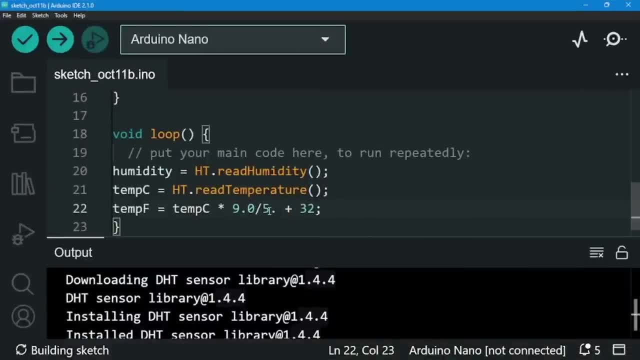 I want to. I want to what? set it to float 9 over 5. there we go. what other problem do I have here? the other problem that you might notice- you might not notice right now- is that what, right here, Arduino does not know. what are we supposed to? what are we supposed to do? this first, this: 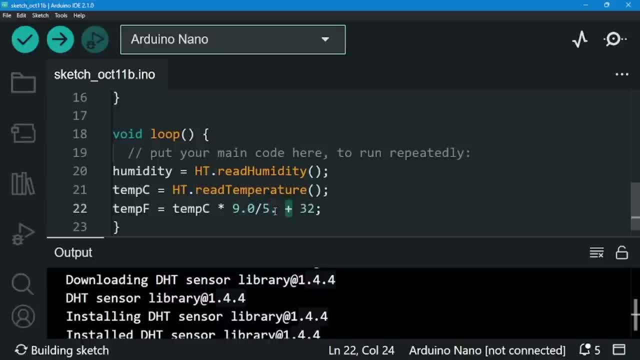 multiplication first or addition first? it does not know what to do, okay, so we're running into another problem right here. should I do the addition or the multiplication first? if it does the multiplication first, what happens? temperature Celsius is going to be multiplied by 9 over 5, and then, finally, it's going to be added by 32. 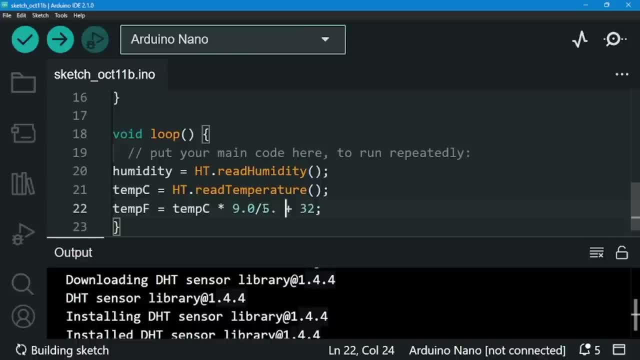 but if we add, if we do the addition first, what are we saying? we're saying, oh, 9 over 5, we're going to add it to what? we're going to add it to 32 and then, after adding it to 32, what do we do? 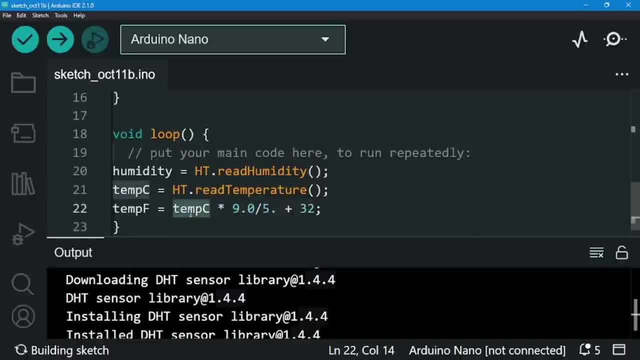 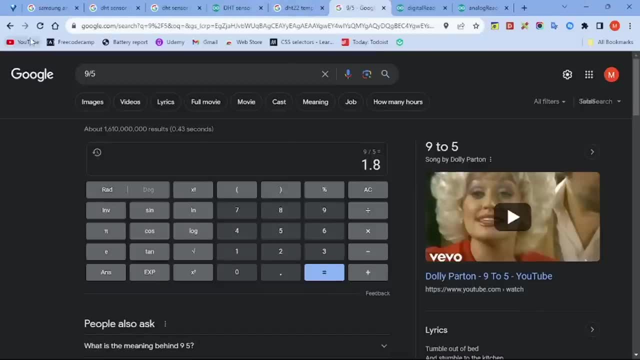 we multiply it to the temperature Celsius, okay. so right here there's going to be some confusion. what do we want to do right here? let me just again look at our code. let me just look at our formula right here. it's better that way. where's our formula? let me just go back. 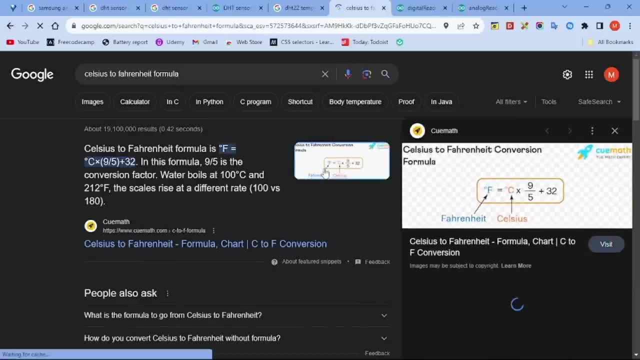 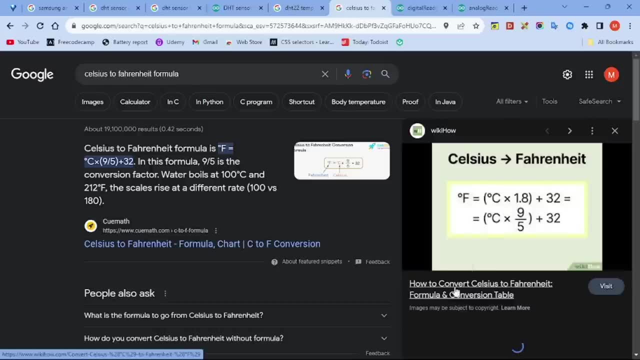 there we go. can you see it? we wanted what we want: to multiply it first and then add it up. okay, we want to multiply first, right here, you can even see it, right here. we want to multiply it first and then we want to add it up. how do we tell Arduino to do that? obviously we need to do, is we need to. 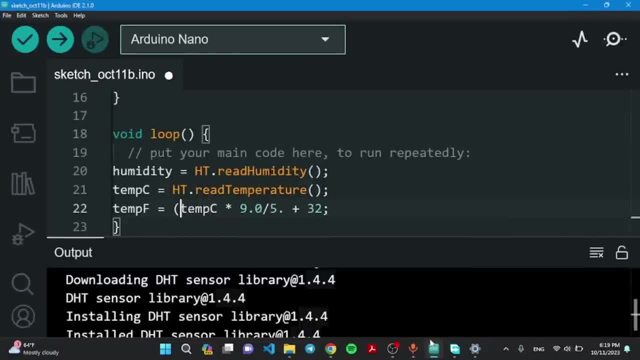 put a parentheses. okay, so let me just put a parenthesis right here, the parentheses. there we go put a parentheses, all of this. so I want Arduino to do what I wanted to do it together. I wanted to divide it first and then divide it by 32.. 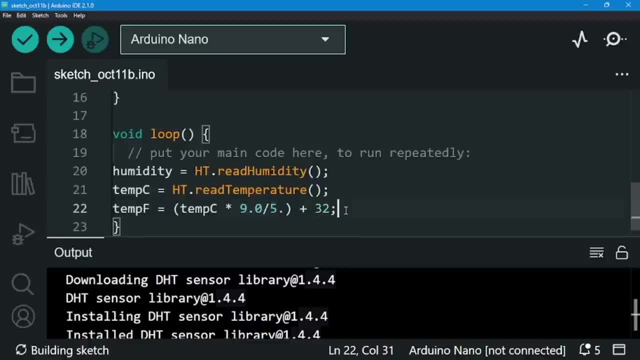 I want it to what? I want it to add 32 as a whole. Okay, then, how do we go to temperature Kelvin? When it comes to temperature Kelvin, what do we need to do? All we need to do is add 273 from temperature Celsius. 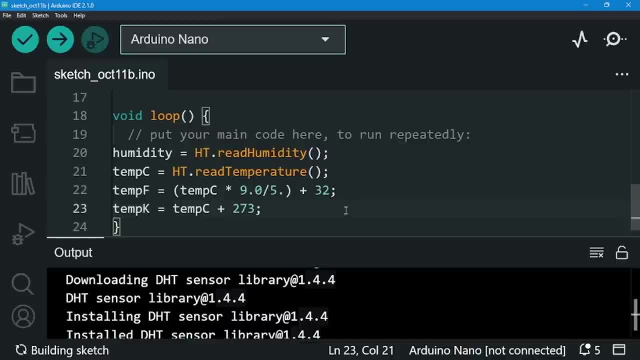 That's all we need to do when it comes to Kelvin. It's very, very easy, Okay, once we're done doing that, actually, it's better to use what? again, It's better to use float numbers. Again, we're using a float number here. 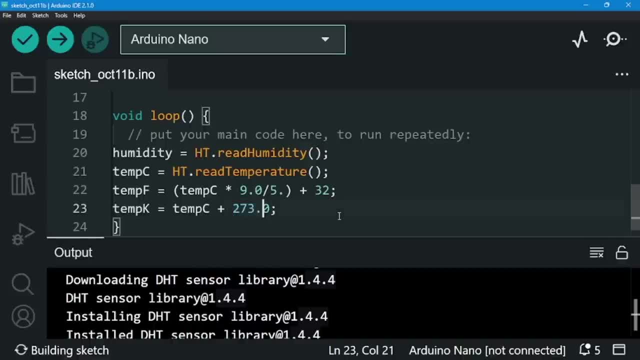 so it's technically best to use float numbers here too, okay, instead of using integers. Okay, then, what do we need to do? That's all we need to do. That's all we need to do. So we found the temperature: Celsius, Fahrenheit and Kelvin. 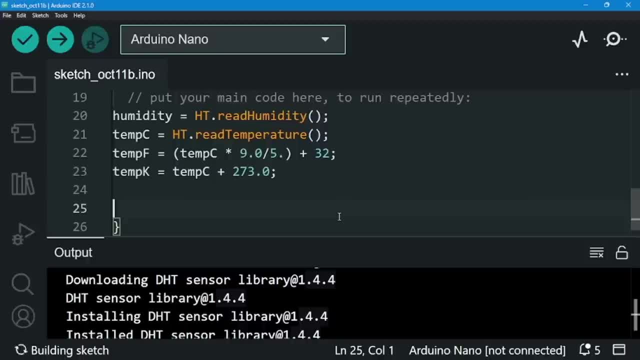 We extracted those information already, Okay, so right here, what we need to do is what? All we need to do is print it out. How do we print it out? We see temperature Celsius. Why are we writing temperature Celsius? You might be asking me. why are we writing it down? 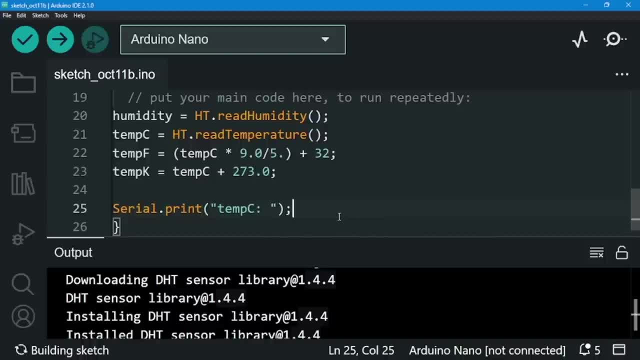 Well, we're going to be receiving three values simultaneously, so we do not know which one's which. So it's going to act as our like. it's going to act as if it's an indicator. okay, So temperature Celsius. 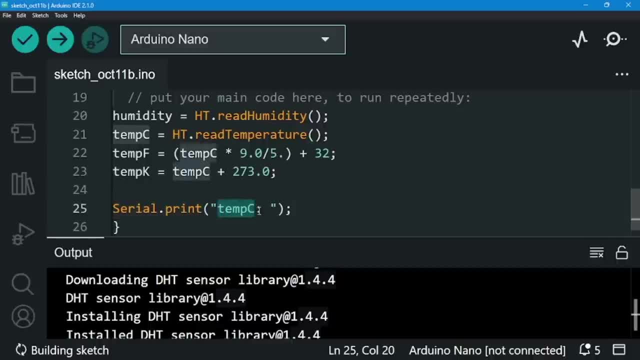 the string of temperature Celsius that's written down as temperature Celsius is going to tell what It's going to be written next to what, Or what It's going to be written next to temperature- the temperature Celsius value right here. So we're going to know which one's which. okay. 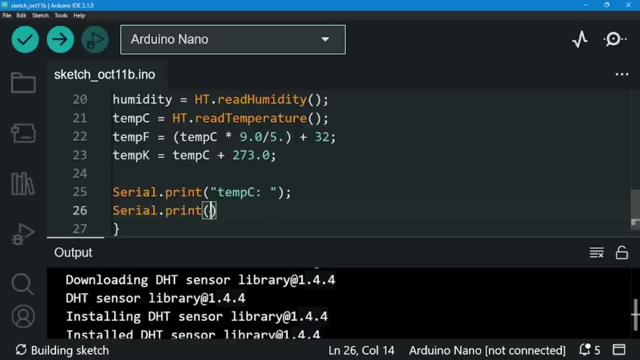 So when we read the value right here, we're going to have three values coming in at once, So we're going to know which one's which. Okay, so I wanted to print temperature Celsius. So I put again an end right here because they're written down. 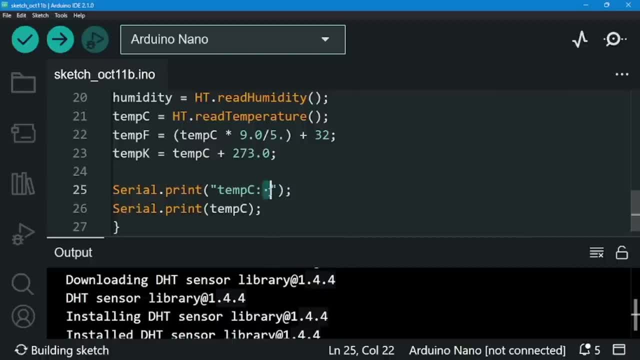 I put a space right here. Why is that I put a space right here? I put a space right here because I'm using what? Serialprint? okay, What happens when you use Serialprint? They're going to be written down in a what? 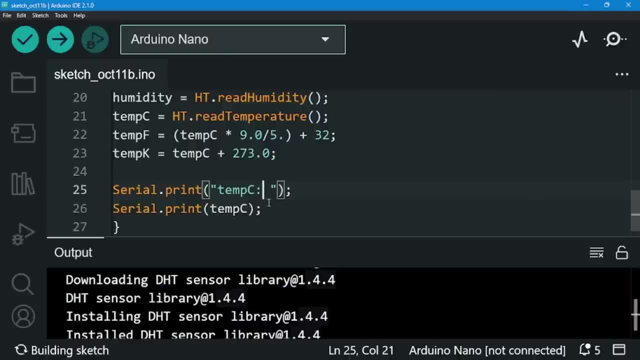 In a one line and it's going to be written down next to each other. okay, So temperature Celsius is going to be here and the value after the space is going to be what The value is going to be displayed. But right here, one thing I want to do is what. 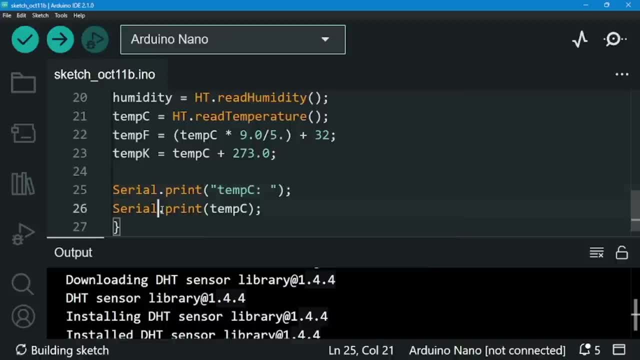 I want to add it to the new line afterwards. okay, I want to add it to the what in a new line. After it's done doing that, I want it to be in a new line and then I want it to print again: Fahrenheit and then Kelvin. 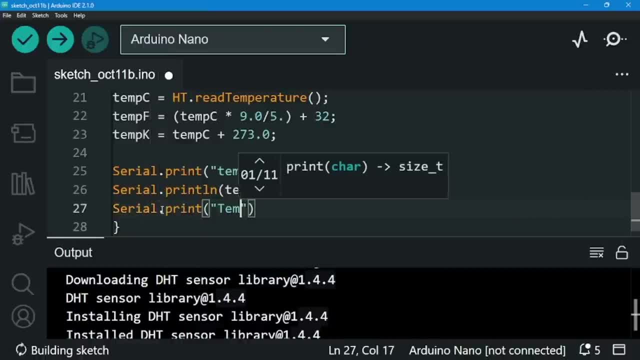 So let me just do that: Print and then set temperature Kelvin. That's all I need to do. It's almost copying code right now. Temperature Kelvin. Actually, wait, let me do temperature Fahrenheit first, because I set it up like that. 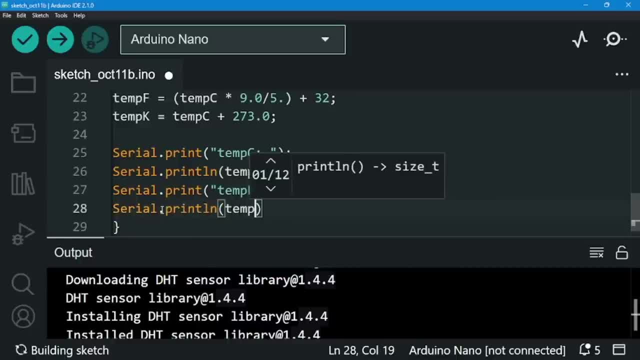 so it would be more fair to do it this way And then write down temperature Fahrenheit. What do I need to do afterwards? It's temperature Kelvin, And then print it in a new line again: Temperature, what The Kelvin temperature? and then it's best to give it what. 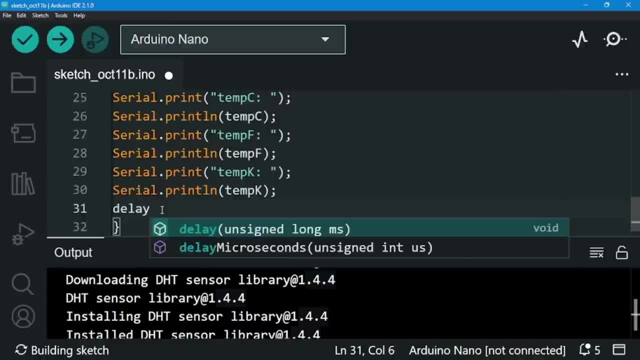 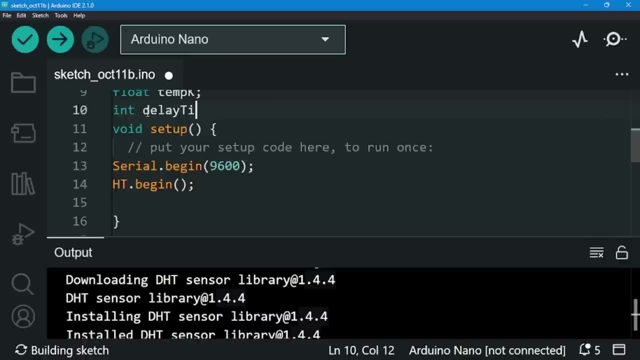 A delay after reading it, so you can again give it a delay and set a delay time right here. Let me set up a delay time, Let's say integer delay time. Let me set it up right here and set it to, let's say, for us to read it. 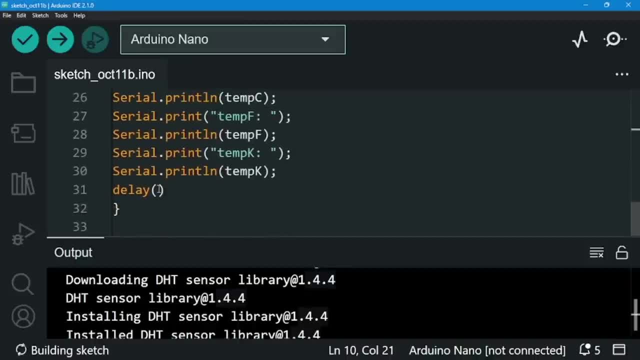 let's say 300 milliseconds, so we can read it properly and put a delay of 300 milliseconds. Okay, That's all we need to do. So right here again, all of this code again is pre-written for us and it's already what the library covers, everything for us. 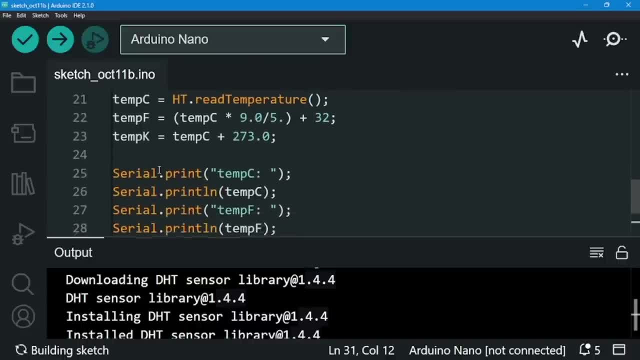 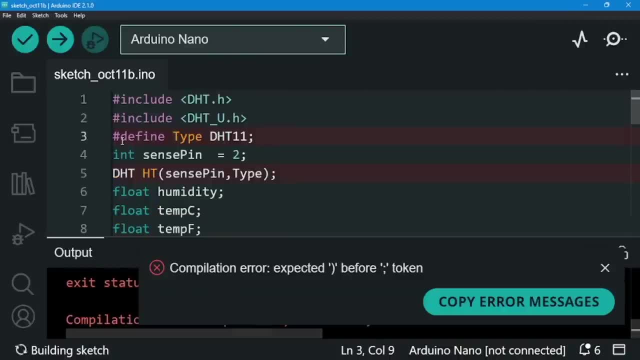 so all we need to do is not even understand how even the DHT sensors work. So let me go back to that's all we need to do actually. Let me just upload this. Let's see if it compiles properly. Expected what. 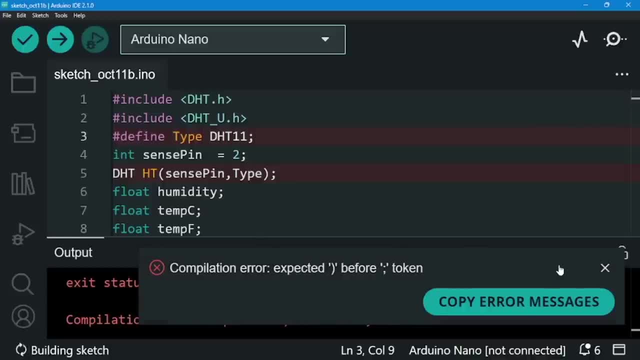 Expected what? What is this saying? What's it saying Expected? oh, parentheses before these tokens. Oh yeah, I'm not using anything here. Did I do anything wrong? It's saying that I should use a. it's saying that I should use a semicolon at the end. 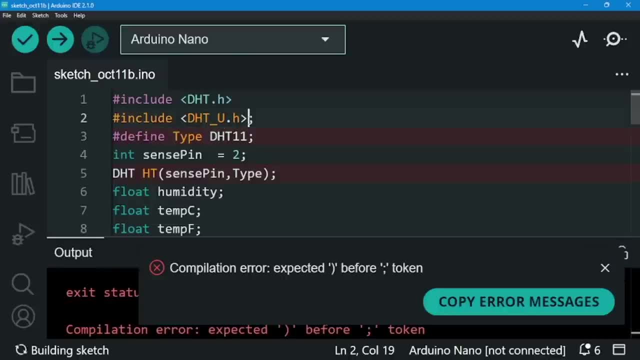 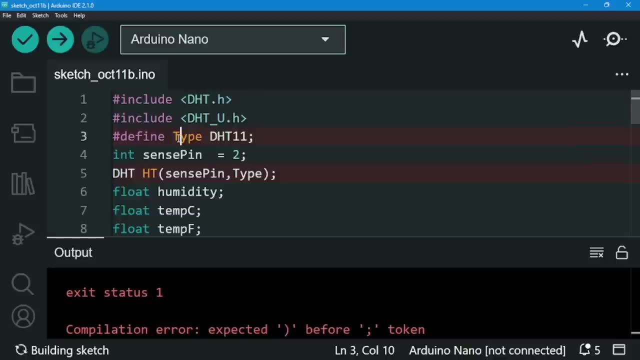 but I don't think that makes sense. It's going to even give me an error right here, And it's going through an error right now because I don't have my Arduino. But for those of you again who have your Arduino and you hooked it up and all, 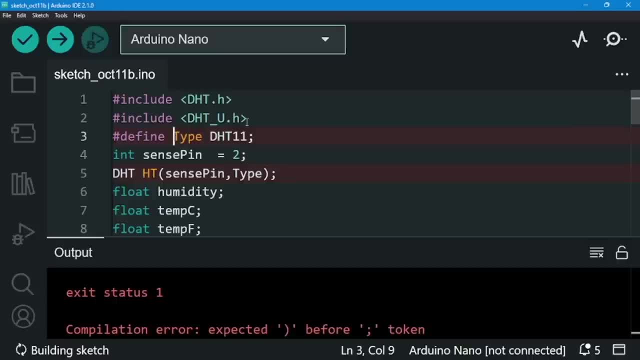 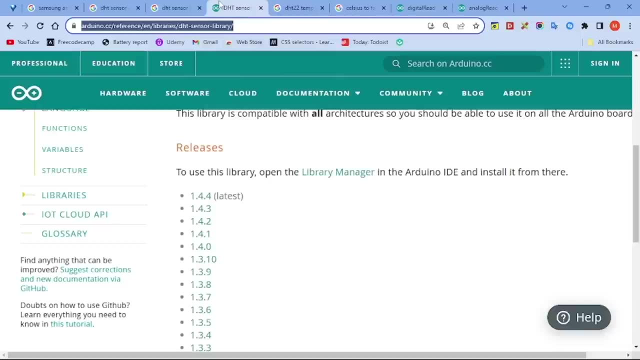 it's going to be perfectly working fine, all right, So just keep that in mind, Okay. So one thing I want you guys to keep in mind is: right now, it's going to be working perfectly fine for you guys, for those of you who have a DHT sensor. 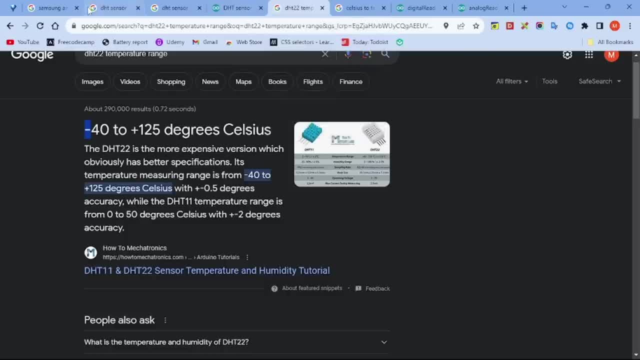 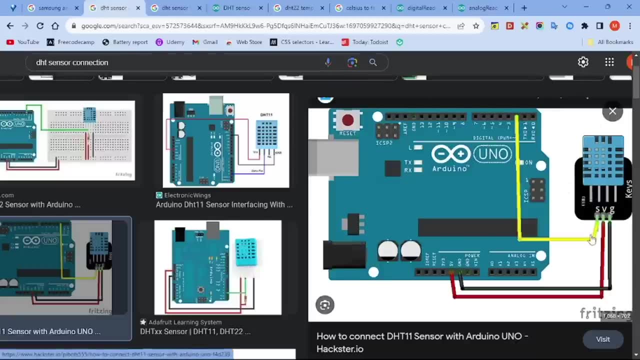 One thing I want you guys to keep in mind is when you're using DHT sensors is- let me go to my connection right here- And one thing the DHT sensor does is it sends out signals of zeros and ones really, really fast. 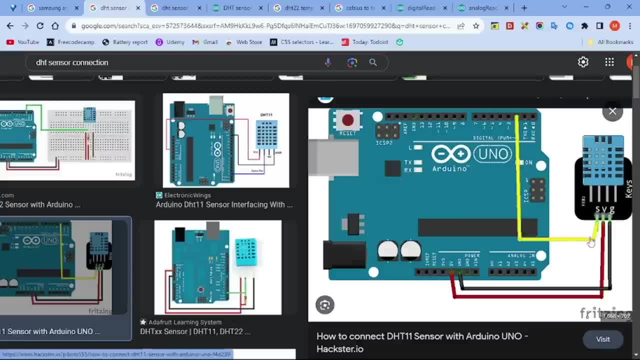 I'm talking zero one, zero ones. It's going to be sending out what bits of zeros and ones. It's going to be basically saying: zero means what, zero means off and ones means on. So it's going to be sending that very, very fast. 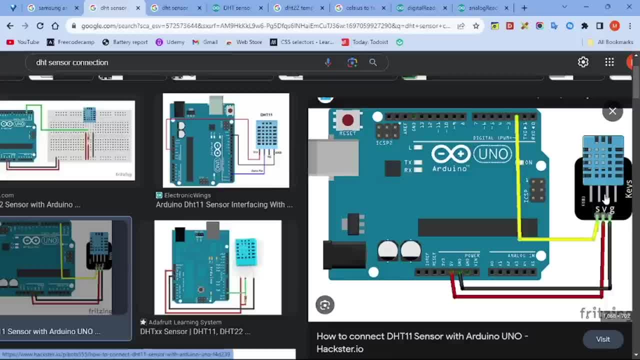 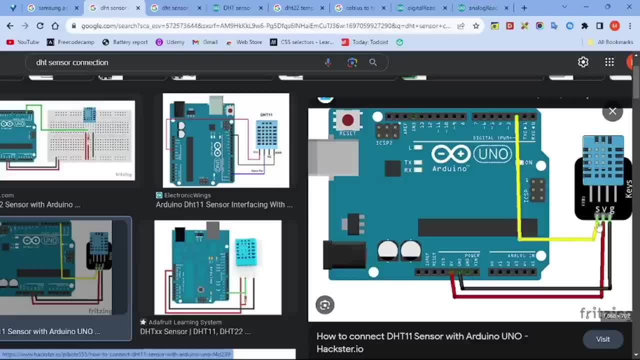 It's going to be sending that through the what, Through the, again, the yellow wire right here which leads to what? Digital pin two. So it's going to be sending what? Again, it's going to be sending zeros and ones, zeros and ones. 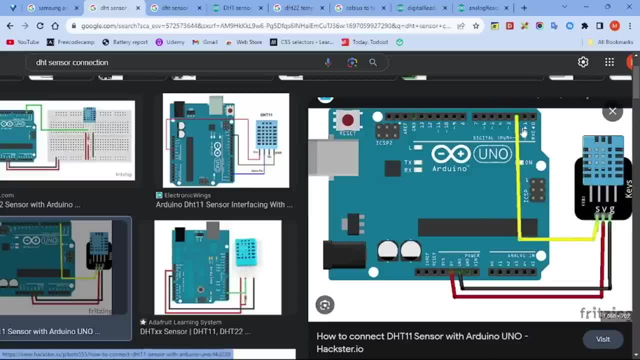 And then our Arduino is going to be interpreting that. all right, It's going to be interpreting that. It's going to be interpreting the zeros and ones. Okay, So it's going to either output zero and one, So it's going to be interpreting that. 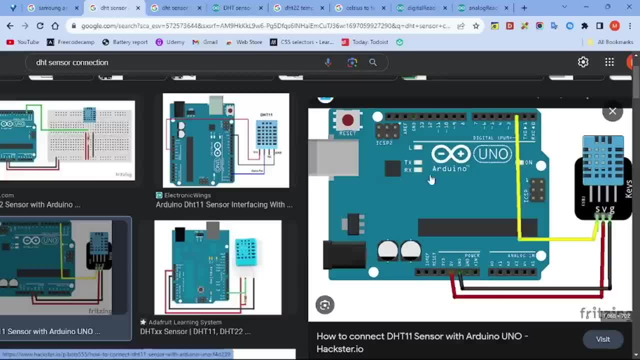 And then it's going to what It's going to again. write it down and print it to our- what? To our serial monitor. Okay, Obviously we cannot see. we're using zeros and ones. How do we read zeros and ones in Arduino? 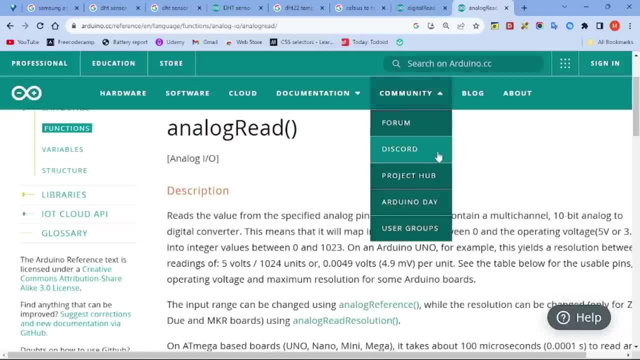 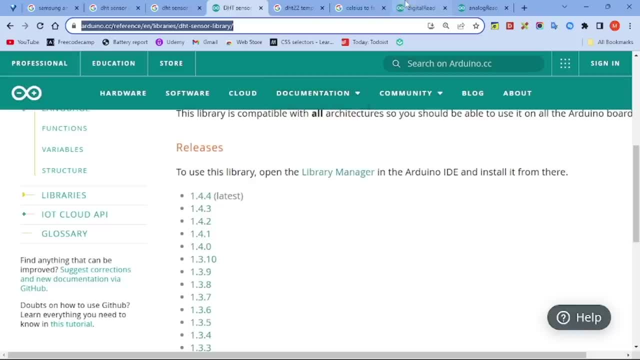 How do we do that? We use analog read, right, Because analog read lets us use any value from zero to 1023.. So when you're reading something, we use what We use analog read. Okay, But obviously we're using what. 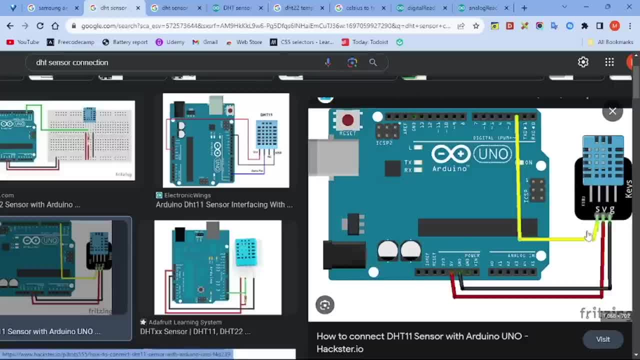 We're using libraries, So, again, it's going to be the library is going to be the one that's going to be doing the, the analog read, right here. Okay, That's one thing I want you guys to keep in mind. 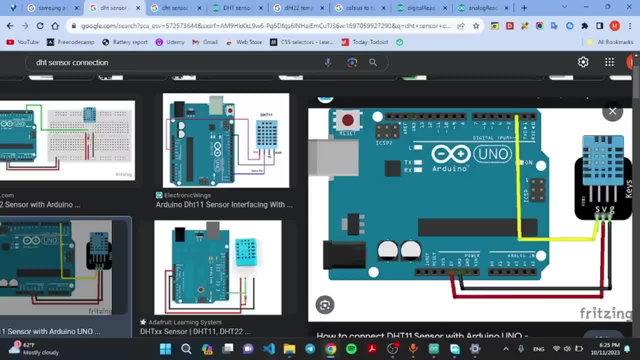 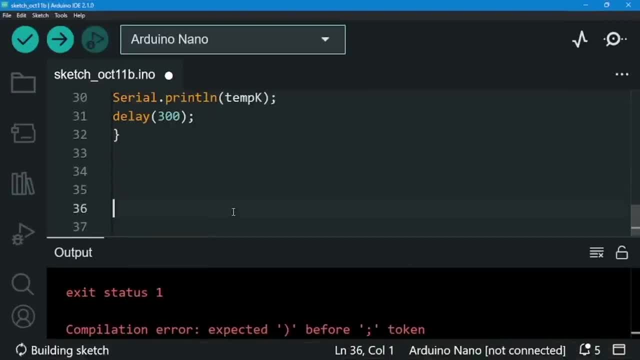 So why do we use that digital pins instead of analog pins? So let me go right here and I think let's go with something more familiar with you guys. So let me go all the way here and let me try to explain this right here. 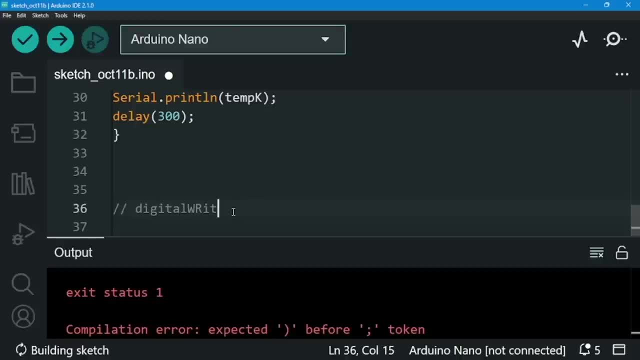 So, when it comes to, if you remember, digital write, what values did it give us? What was the outcome of digital write? It was either high, which basically meant what It basically meant- five volt- or on right, When it came with the other options. what? 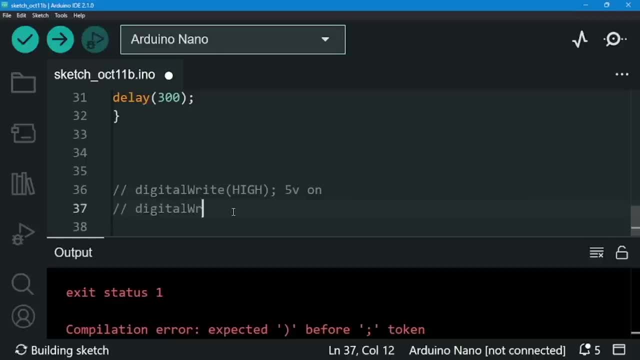 The other option was what The other option was: write it down properly. It was low. What did it mean? Digital write low meant what? It meant zero volt or basically what Off Basically meant off. So there's like two outcomes to what. 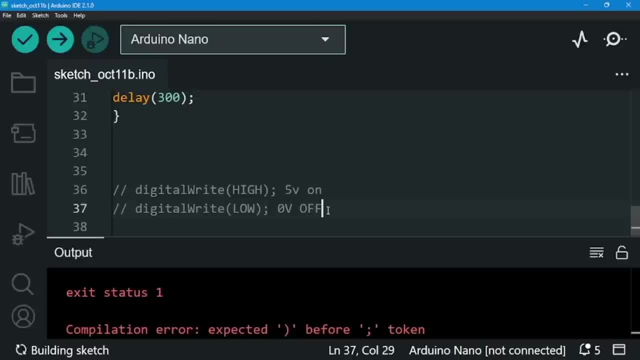 To digital write, Similarly, as we have digital write and we have digital write- right here Digital write- And then we have analog write. We have analog write. Okay, We do have both of them, But we also have, as we have, analog read too. we're familiar with analog read. 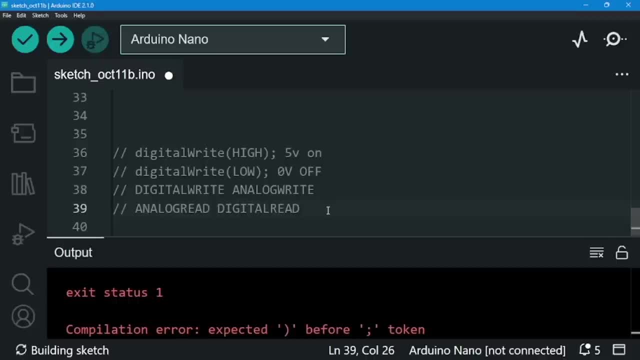 We also have something called digital read. Okay, So what does digital read do? Digital read, what it basically does is you can read the documentation for yourself, But it's going to give us what Information right here. So digital read does is what 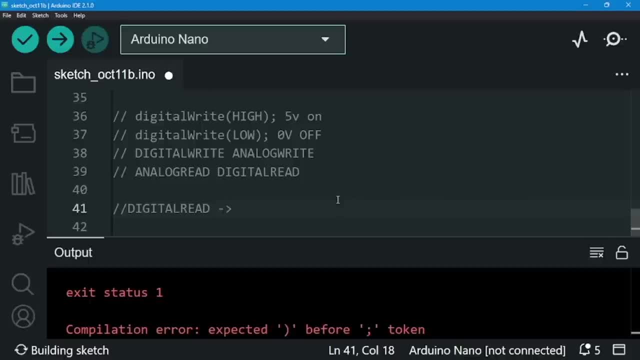 It tells us, if it's either, what? If it's either zero or one? It's going to be telling us. if it's either zero or one, What does this mean? It's going to be telling us if it's zero, it means off. 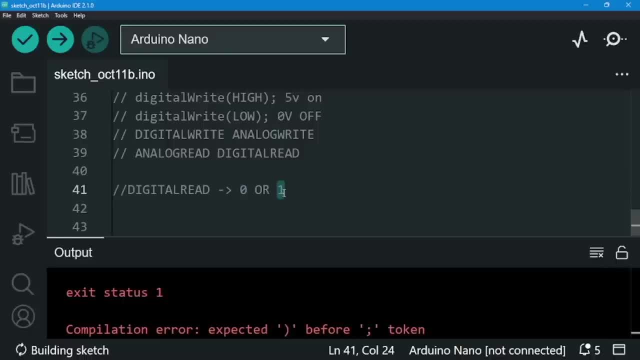 Or if it's on when it's one. Okay, So it's going to be telling us that, So it's going to be telling us if it's on or off, On or off. That's what basically digital read does When it comes to analog read. one thing- that again why you shouldn't be using analog pins- is we have 10 bits of information that is being transferred. 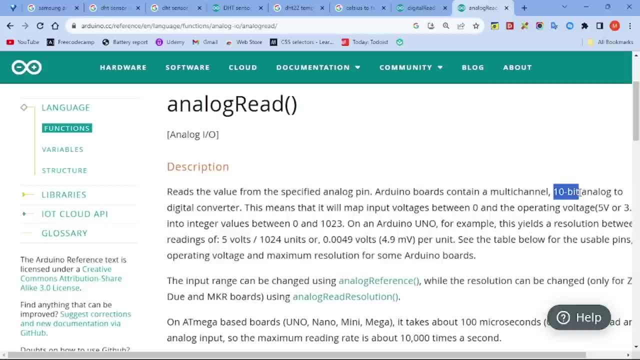 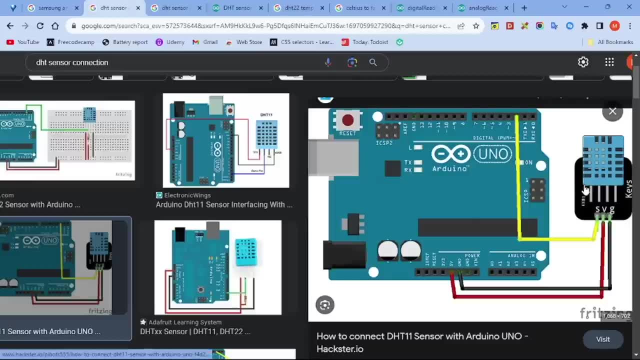 10 bits is a what, It's a bigger number, It's more options. Again, it's useful again, But right here it's not Because, as I said again, our, again, our Arduino, our, there we go. our DHT sensor always sends zeros and ones. 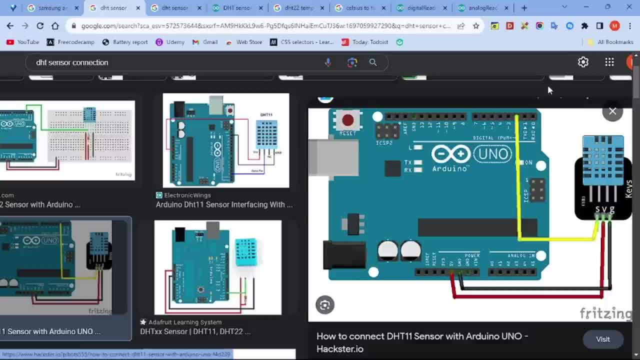 Bunch of zeros and ones really really fast. Okay, So it's going to be either zero or one That's going to be sending, but it's going to be sending it a very, very fast, And then the Arduino is going to be interpreting that. 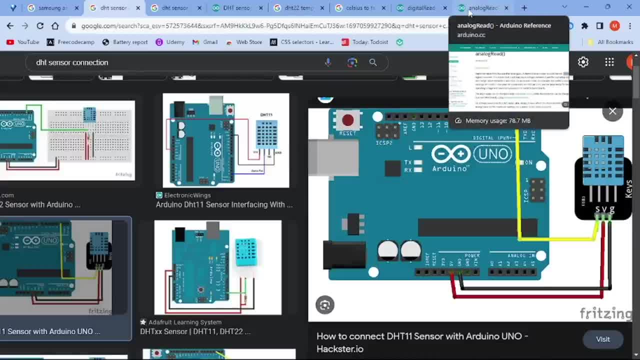 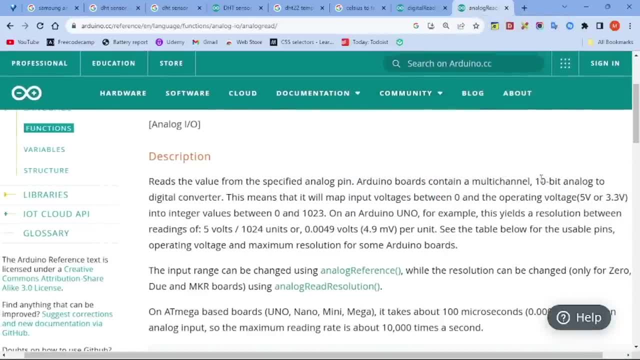 Okay, So the number of zeros and ones again inside of, again the full information is going to be affecting. again, it's going to be telling us our temperature. So right here it's going to be sending out 10 bits of information. 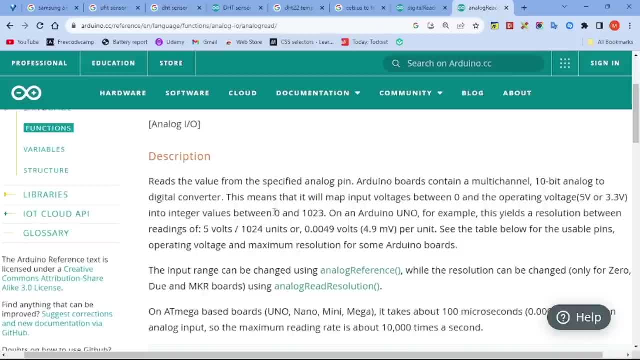 So what happens here is there's what it gives us: a value between zero and 1023.. It gives us lots of options, But what happens here? The limitation right here Is what? basically, what happens is what you only want: zero and one. 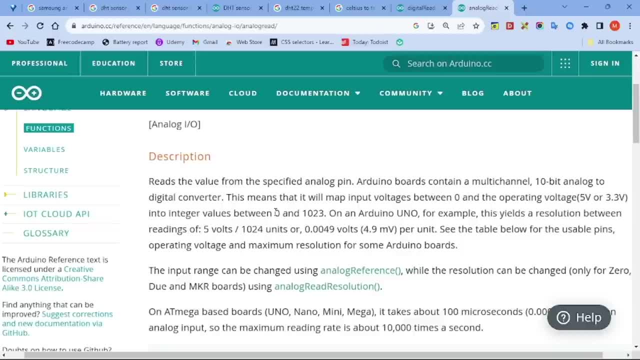 We only want what zero and one, because again, as I said again, are what our DHT sensors are only going to be using: zero and one. They're also, they're always going to be outputting what zero or one on or off. 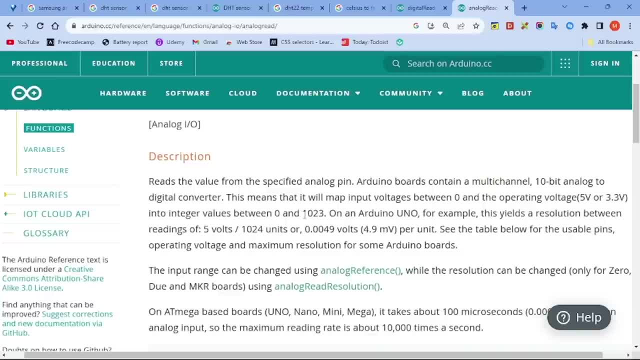 Okay, So they're not going to be using this rest of the value right here, from 1023, anything from what. they're not going to be using anything from two to 1023.. Okay, So it's going to be 10 bits of information always being sent out to what, the Arduino, 10 bits of information being set up to. 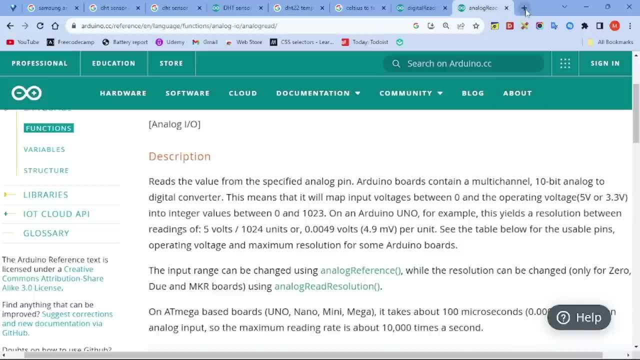 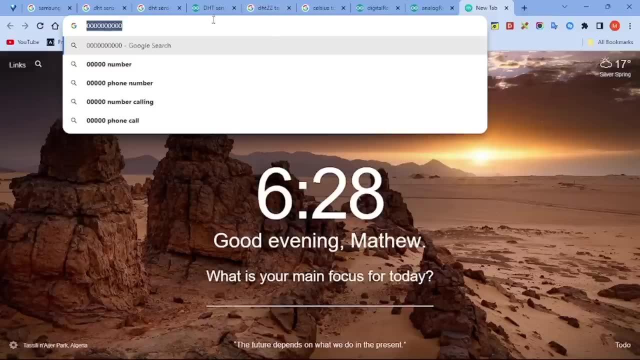 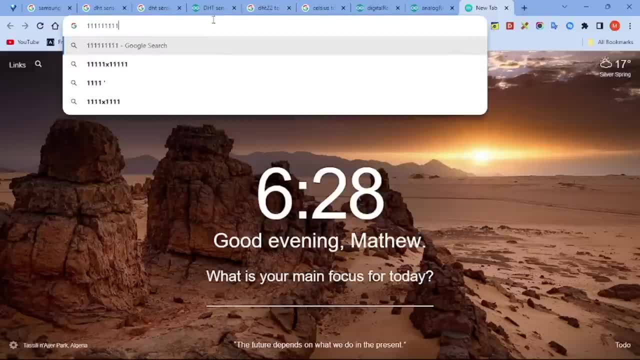 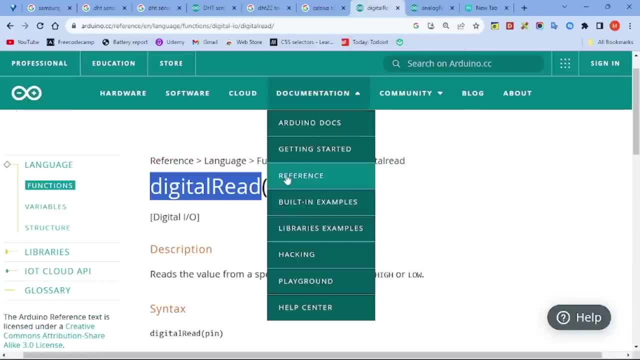 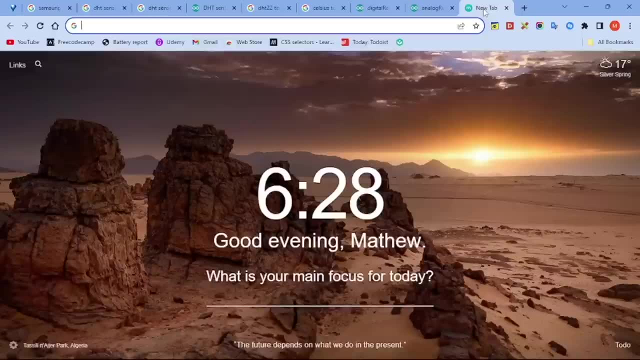 Okay. So when it comes to this- the read right here- we only need what we only receive zero or one. It's going to be sending it in one information: When we have one bit, what's the one bit of zero? It's zero in of itself. 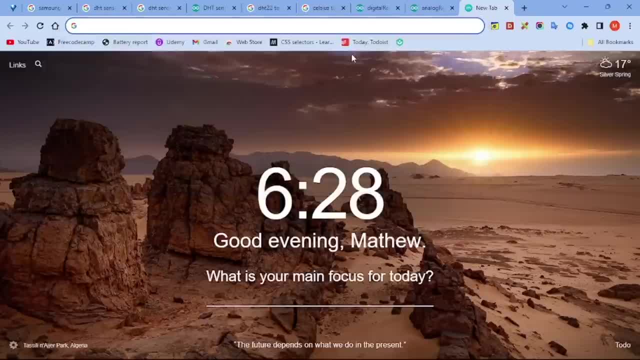 What is the one bit of one? It's one. What's the one bit of two? It doesn't exist. It can only count up to what, can only count between zero and one. Okay, So that's one thing I want you guys to keep in mind. 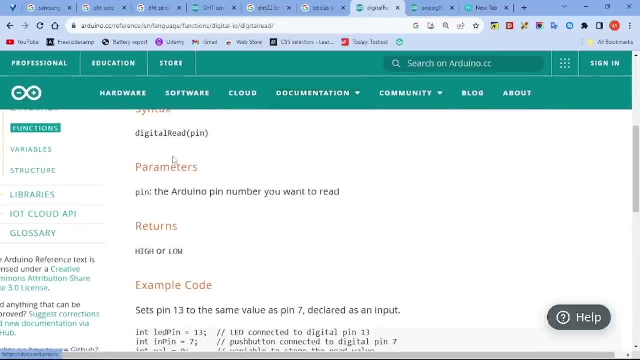 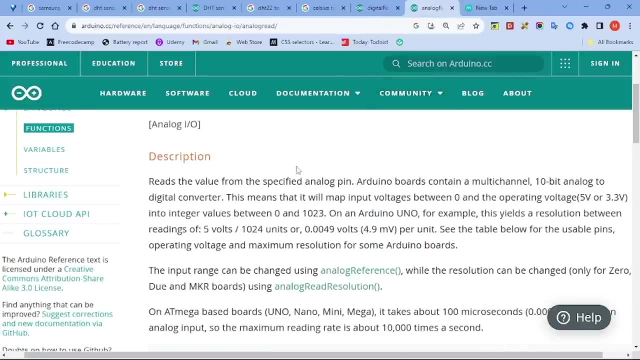 So right here, it's more efficient because it only sends out what? it sends out little bits of information. It sends out one bit compared to the what, compared to the analog. So right here, the analog is going to be sending out 10 bits again and it's going to compound. 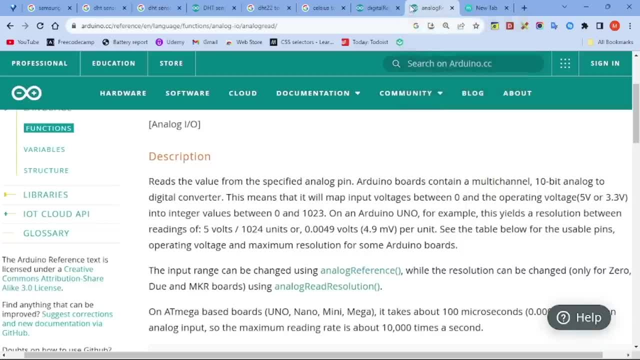 Okay, So it's going to be sending out zero, zero, zero, zero again. one, one, one. So one thing I want you guys to think about when it comes to bits is like how we have conversations: Okay, So 10 bits. what can it do when it comes to 10 bits? 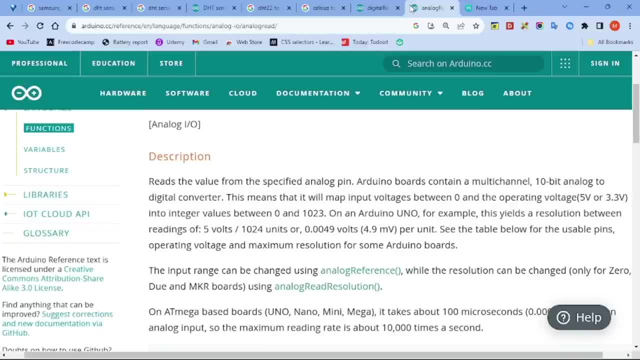 10 bits again. allow us to what? To access different amount of numbers, lots of numbers, Just like. just think of me saying, hey, how are you? And just think of it as being 10 bit. Okay, Hey, how are you? is what? 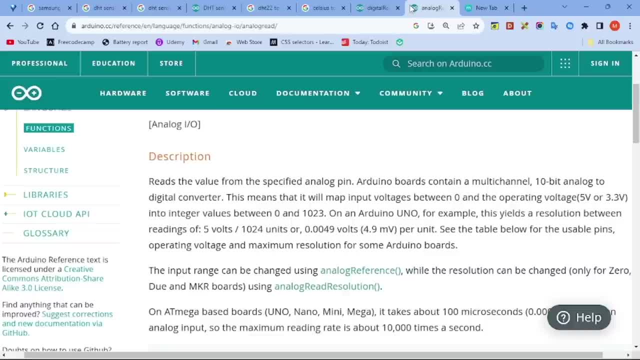 10 bit And think of high. It's what It's, just think of it as one bit. Okay, Which one is faster to say? High is faster to say. Why is that? So we're transferring a smaller amount of information. 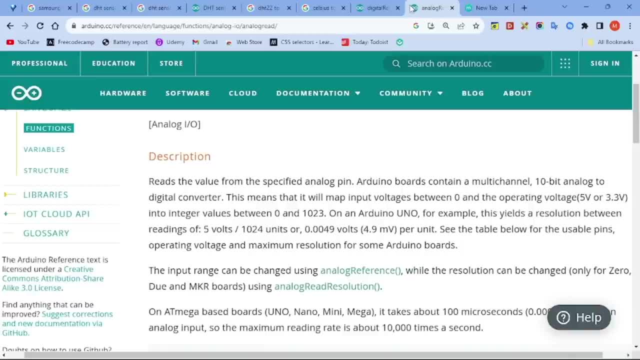 Okay, We're transferring what Smaller amount of information right here, So it's faster. So the problem here is what? The problem with analog read is it transfers 10 bit. Okay, It transfers 10 bit, and it's going to be what? 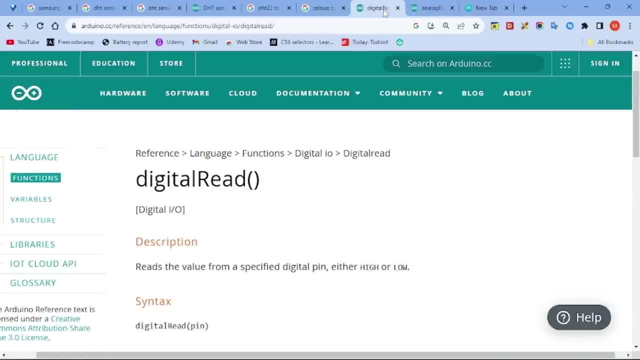 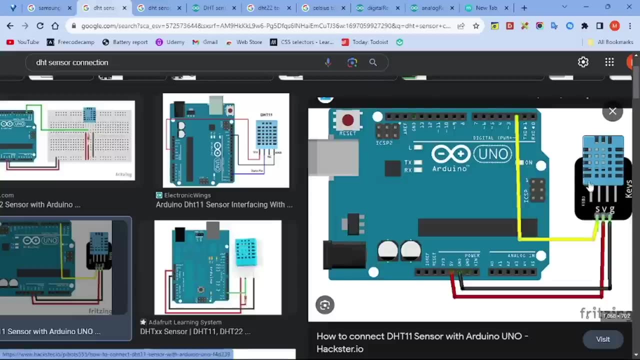 It's going to be slower when it's compared to the what, To the digital read. That's why it's preferred to what To use digital pins when it comes to this again, DST sensors. I want you guys to keep that in mind. 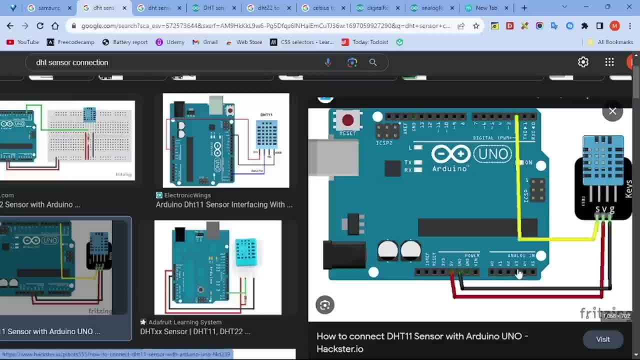 Yes, you can use analog pins, but it's going to be what Less accurate, And then also you risk what? You also risk it being slower. But when it comes to the digital pins, we only transfer again one bit of information. 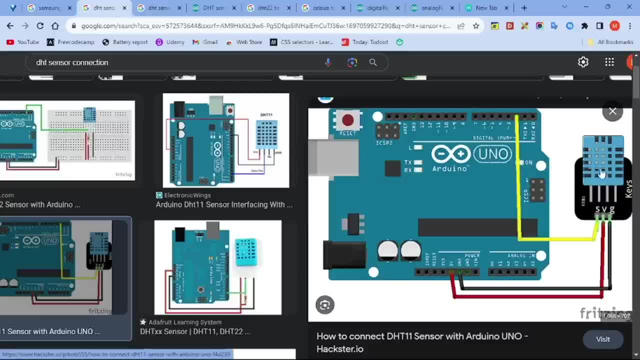 So it's going to be really, really fast because, again, our DST sensor is going to be sending out zeros and ones, and digital read is going to be very, very fast. Again. when it comes to what? When it comes to the digital pins? 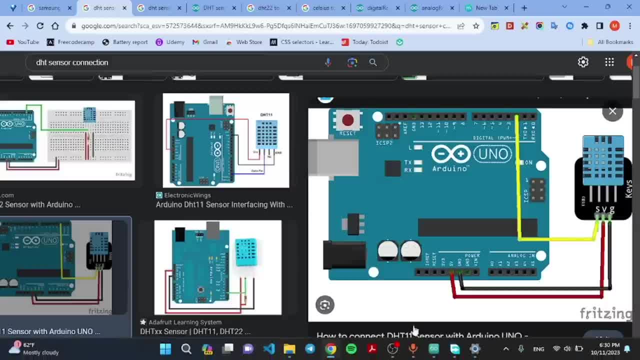 So just keep that in mind. Anyways, with that in mind, everything should be working perfectly fine for you guys. For those of you who have it, it's going to work perfectly fine And you can upload the code and you can work with it. 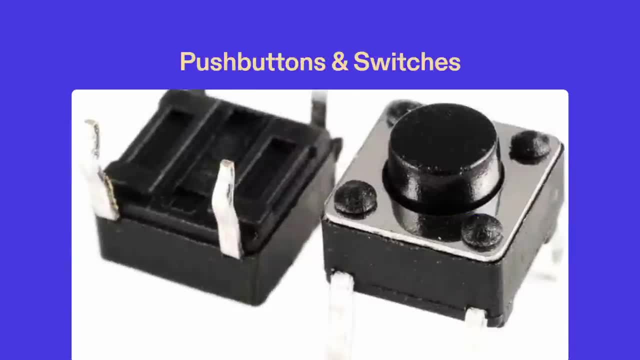 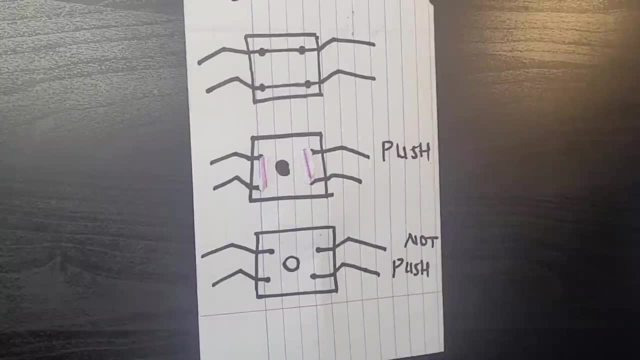 Anyways, with that in mind, let's move on to the next section. In this section, we're going to discuss about switches. So this is going to be a very quick and a very short section, but it's going to be an important section. 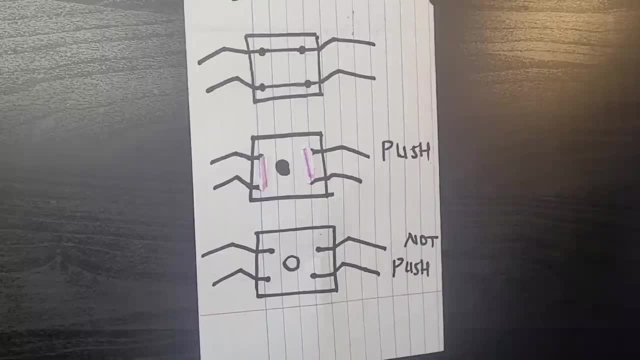 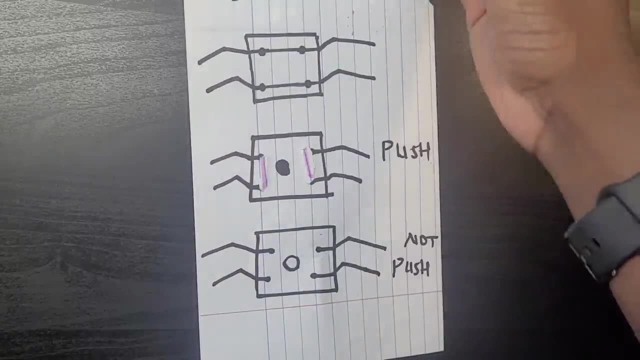 because we're going to be discussing one of the most important parts and one of the most common components that we use in an Arduino- Not only in Arduino, but in our lives. Okay, So today we're going to be Discussing about switches. 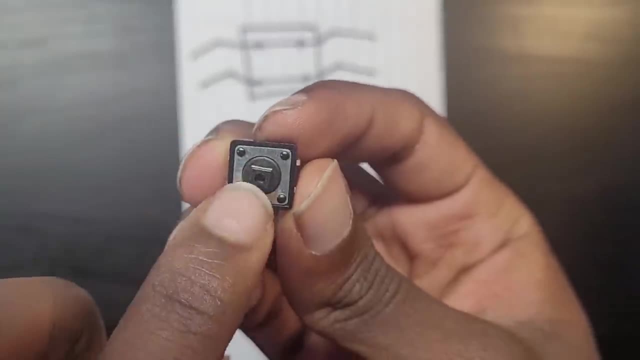 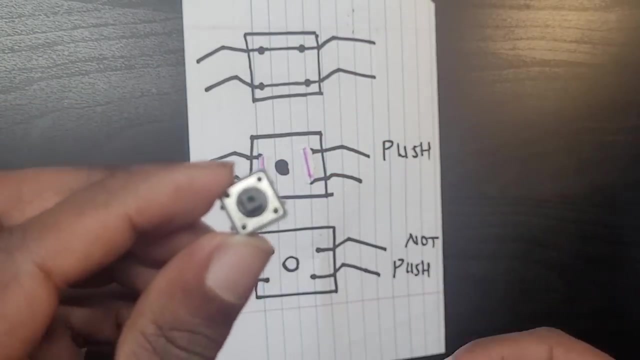 Okay, So switches? they look something like this: They have a button right here that you can push, Okay, And we have four legs. They come in different sizes. This is a big switch, the same type of switch, And this is the same type of switch, but it's obviously smaller. 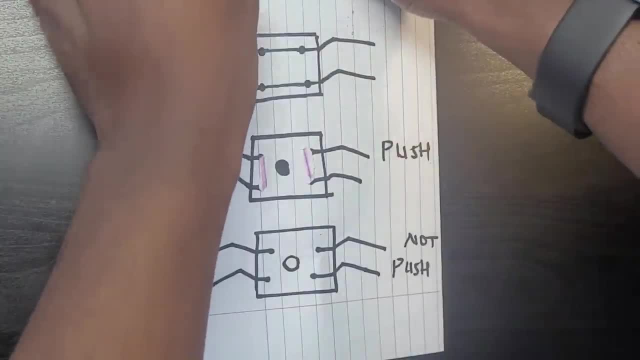 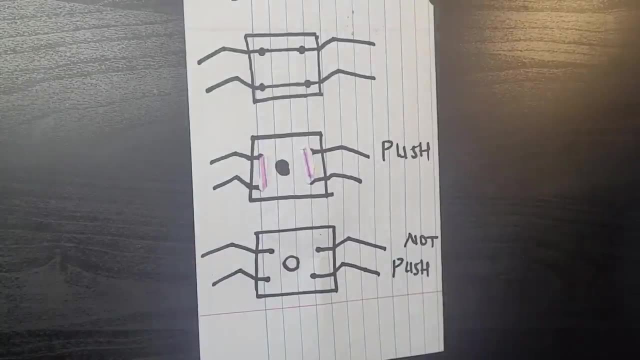 We need to do a side by side comparison, Okay. So one thing we need to understand about switches is they're fundamentally very, very easy. They're fundamentally speaking, They're very, very simple, Okay. So, before discussing about you know, all these switches and stuff- 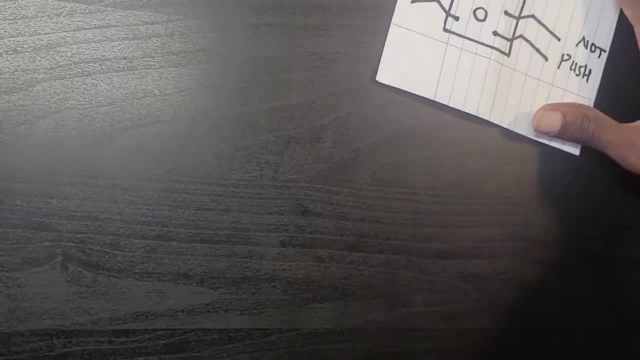 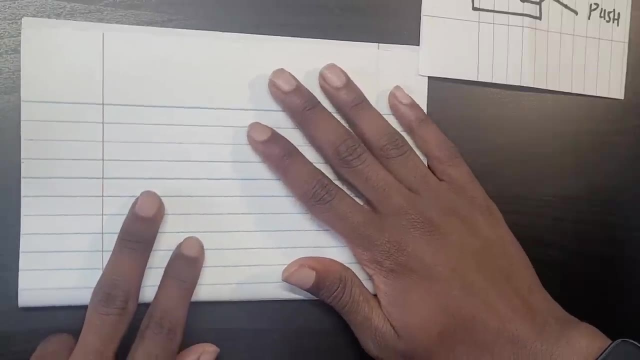 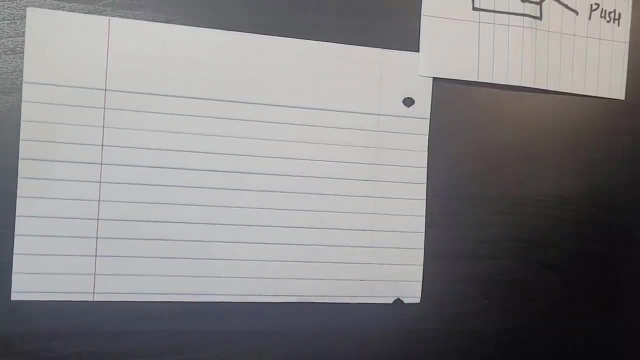 I'm going to get back to this. for doing that, I think it's best by discuss about current right here, because it makes sense to do So, because switches are used to do what switches are used to turn on or turn off something. So turn on and turn off a circuit. 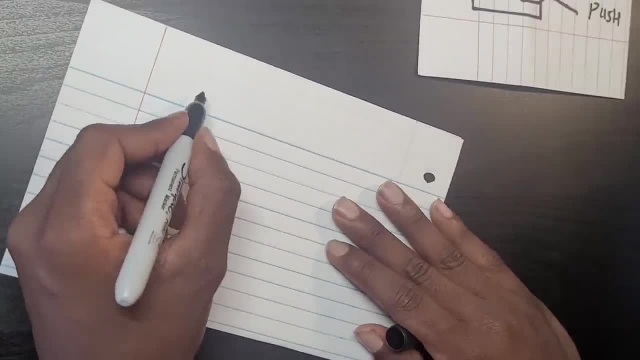 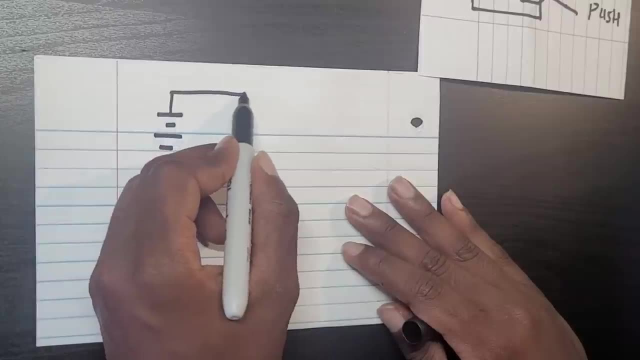 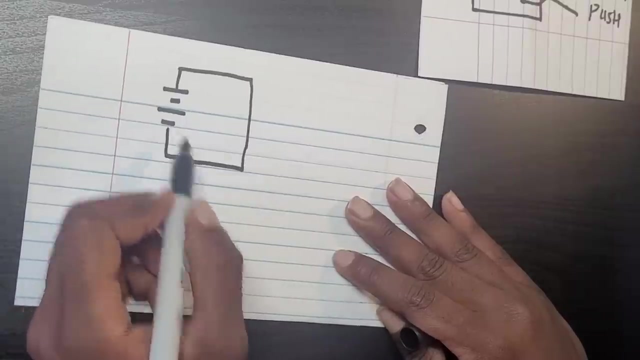 All right. so let me go right here and let's just again create a simple circuit. Okay, let's just do that. This is what? almost a complete circuit. Why is that So? why is this a complete circuit? Because the positive terminal goes and it touched what the negative terminal. 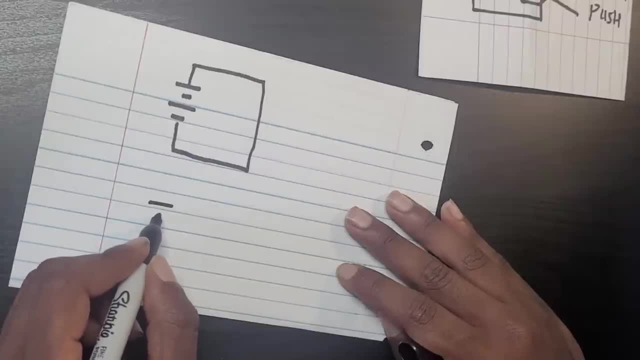 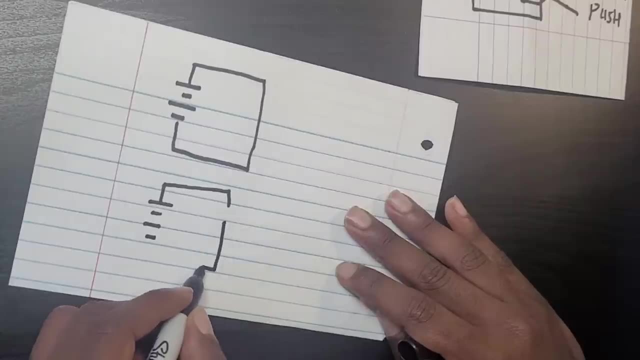 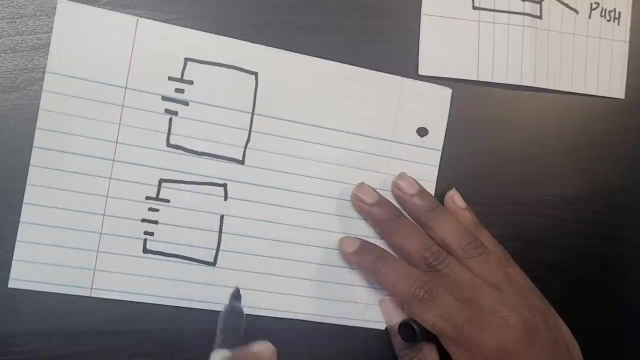 It's a complete circuit. How about if it was like this? What happens if it was like this? What happens if there is an Happening between what? the circuit right here, between the circuit? What's going to happen in this case? Obviously, what's going to happen. 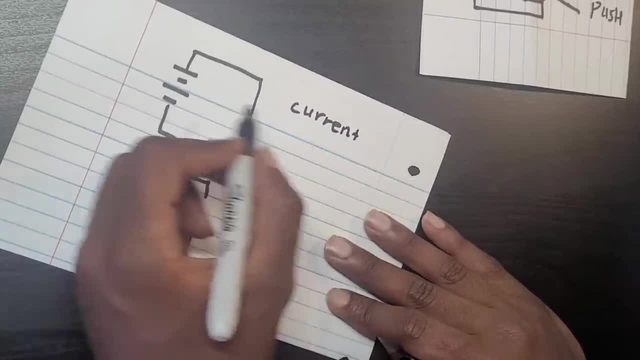 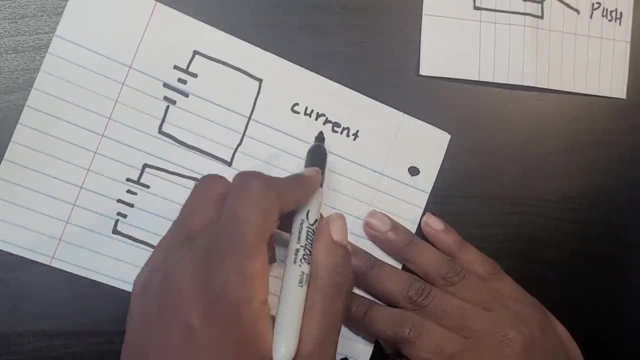 Current is going to flow. by the way, Don't correct connected direct, Don't connect your obviously positive towards the negative, because we have no resistor here. So we're going to fire Arduino. But again, this is just for concept. So current is going to flow. 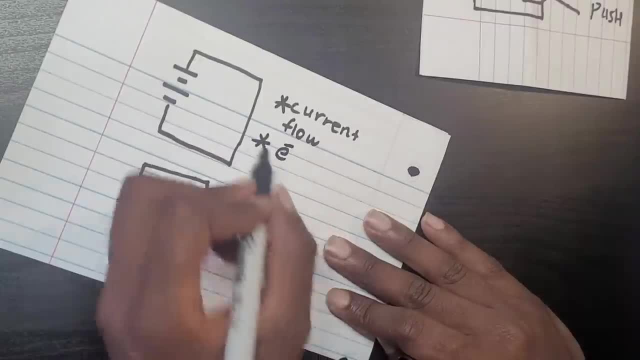 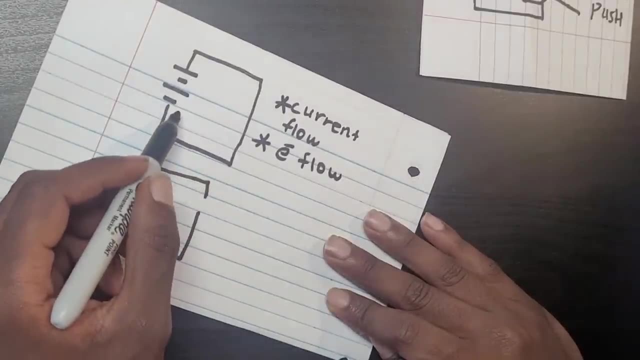 What else is going to happen? Electrons will flow to if current is flowing. electrons are flowing again. currents flow From what position to what position? they fall from the positive to the negative, whatever like trance. they fall from the negative to the positive. They have what opposite Directions? they flow in opposite directions. 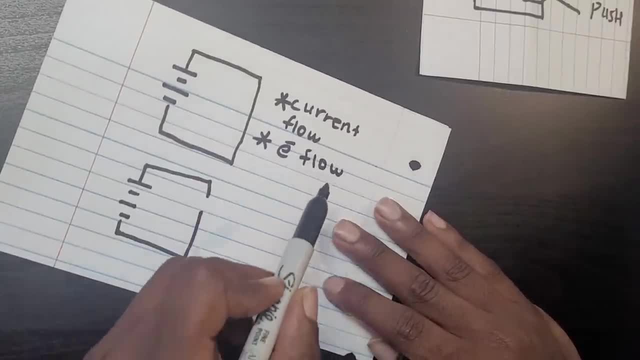 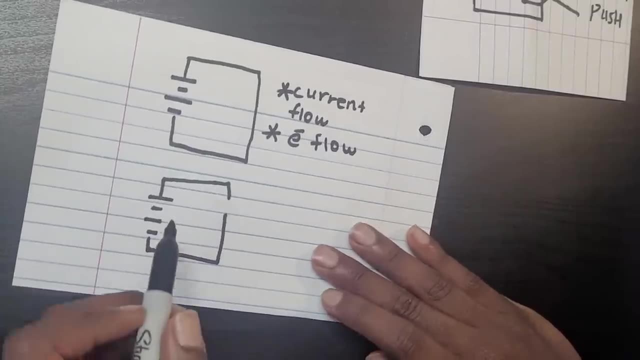 Okay, so obviously you know by now that electron flow is what generates current. Just want you to understand that, Just keep that in mind. Okay, But what happens here? Let's say electrons are again moving from the negative terminal. Electrons are moving. 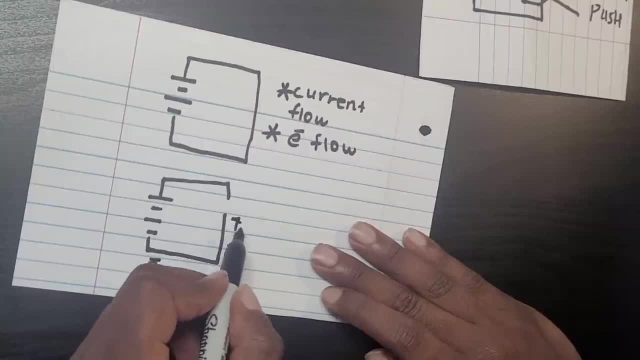 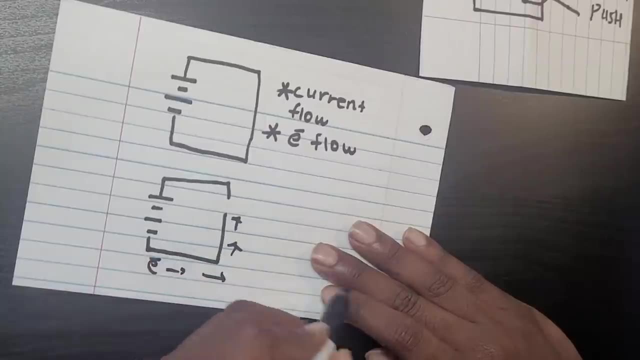 They're moving, They're moving, They're moving here, They're moving and they stop here because they cannot cross this boundary. then what happens here? electron cannot move the whole way. so basically, what's going to happen? there will be no current flow, so current. 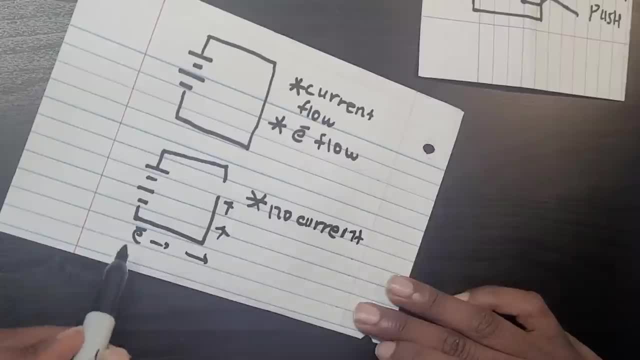 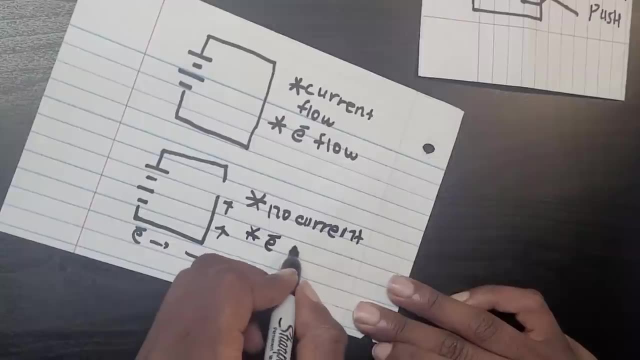 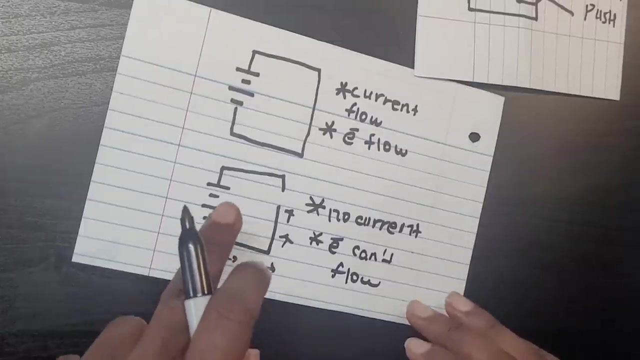 will not flow. because what happens? because the electron cannot flow. from what? from the negative terminal to the positive terminal. so basically, no current flow. because of why? because electron can't flow. because electron can't flow in this circuit. okay. so that's basically the same concept that we're going to be using in switches. so switches, when we turn them on, they make it so. 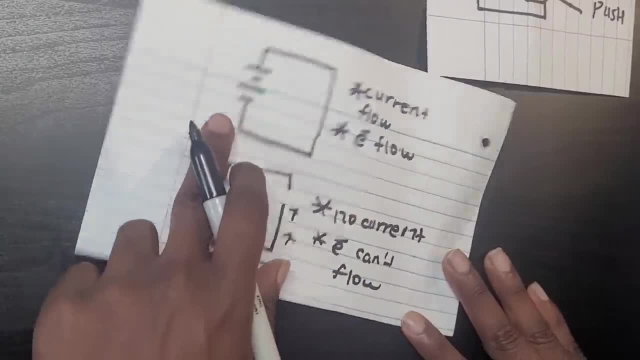 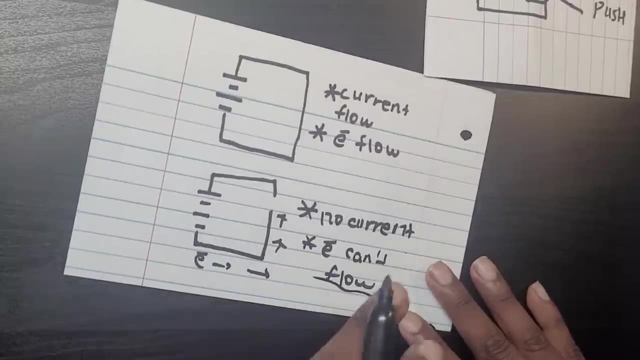 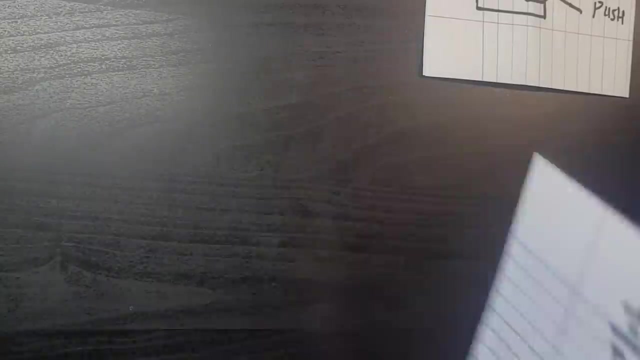 that we can again flow. electricity can flow. can you see it? electricity can flow. but when we turn it off, what do we expect? we make it so that electron electrons cannot flow indirectly, will not have what and will not have any current. okay, so right here, let me just 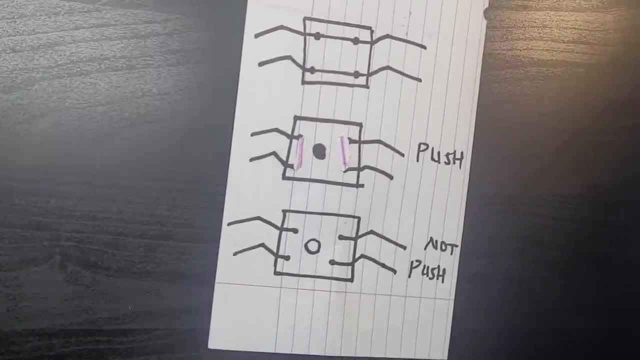 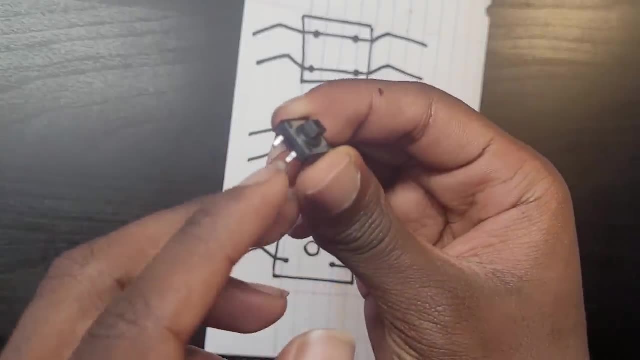 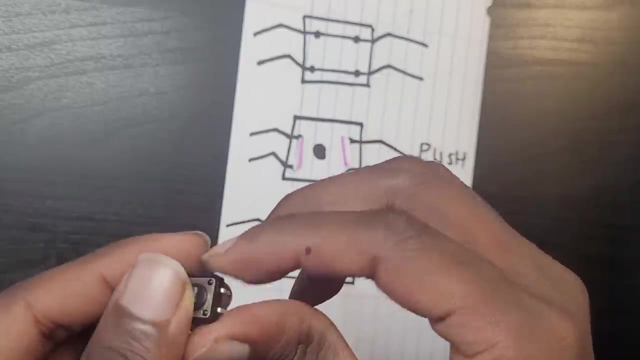 move this. so let me just bring the switch right here. and one thing you want to look in these switches is, again, let me just focus on the switch right now. okay, there we go. one thing you want to focus on the switches is: there are closed sites. can you see this? there are cold sites here, there. 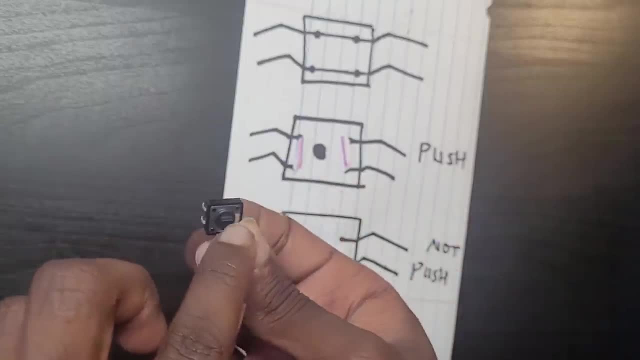 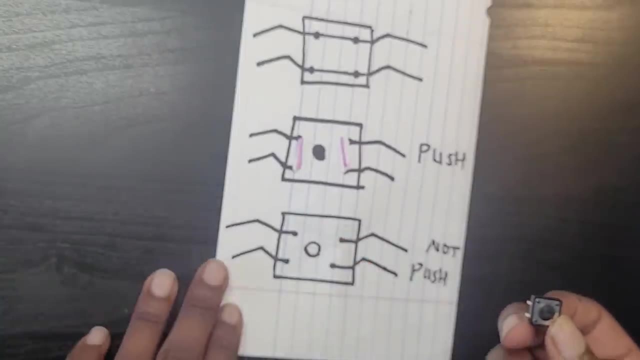 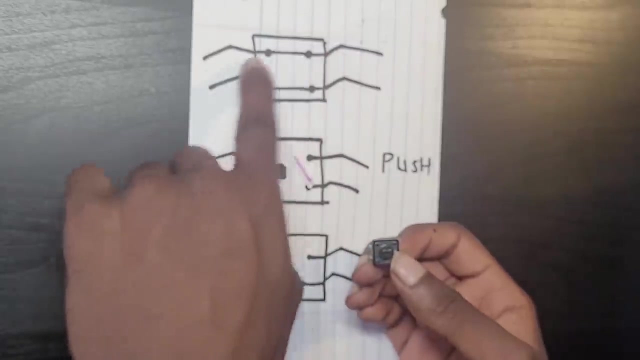 are close sites here too, and there are ones that are what they're connected to, even parallely. they're connected in this direction. okay, they're connected in this direction. so one thing i always want you to keep in mind is the ones that are um, the ones that are facing opposite, the ones that are parallel to each other. 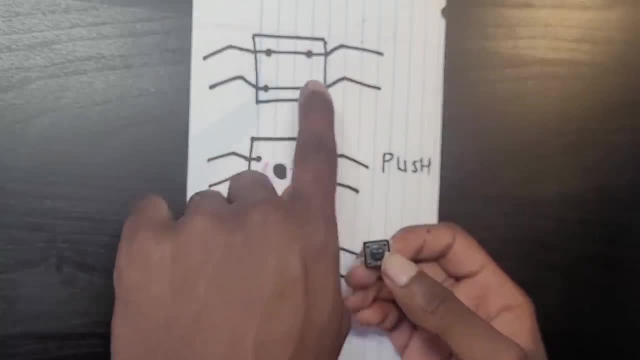 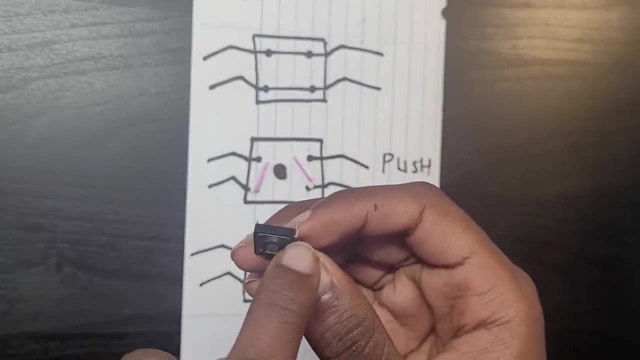 are always connected. i want you to keep this in mind. they're can. they're always connected, either when you, either when you push it or don't. they're always connected, okay. they're always what. they're always connected, okay, when it comes towards, uh, these, these ones that are connected by 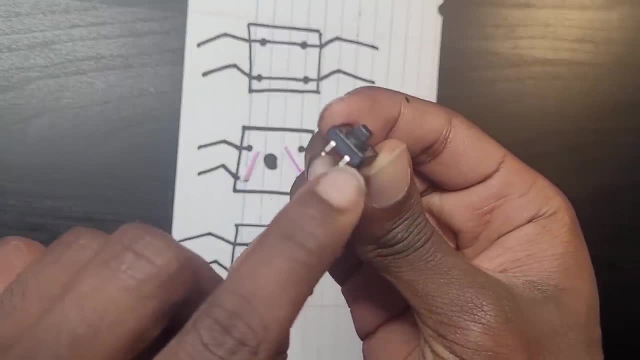 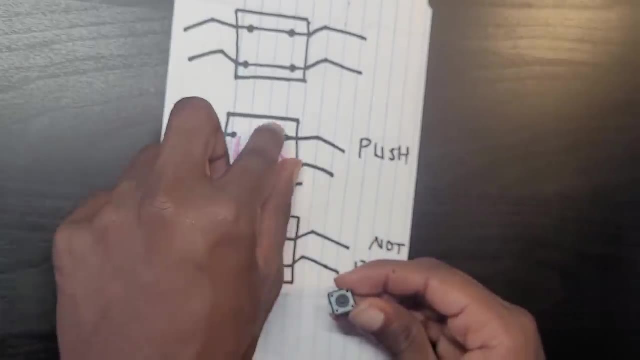 what they're on the same side. so i want you to see the pins that are attached to what the same side. when it comes to those pins, what happens is there are what. they are just gonna put this here. there is a wire, okay, so there's a wire, that's. 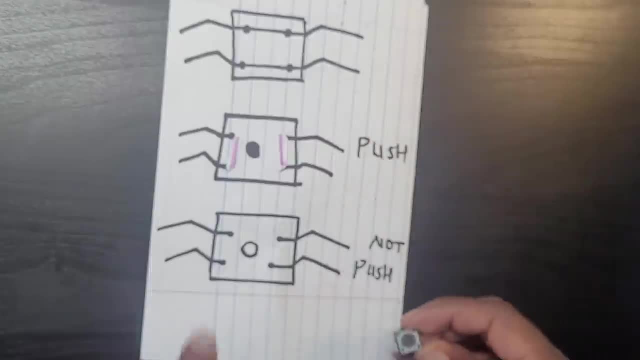 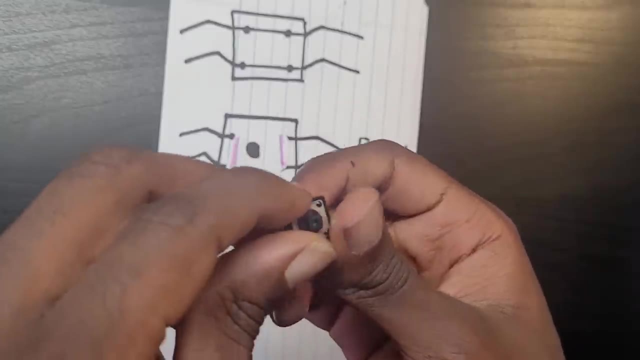 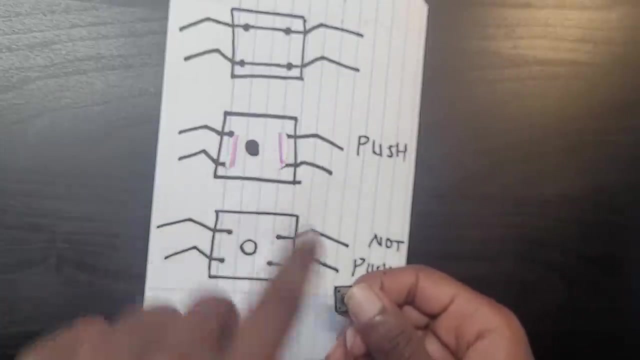 gonna move. it's a wire, that is what that moves, okay. so, right here, when you push down, okay, when it comes to these buttons, when you push down, what happens is, once you do again pay attention- is, when you push down, what happens is these wire attach. basically, when they attach, what happens. 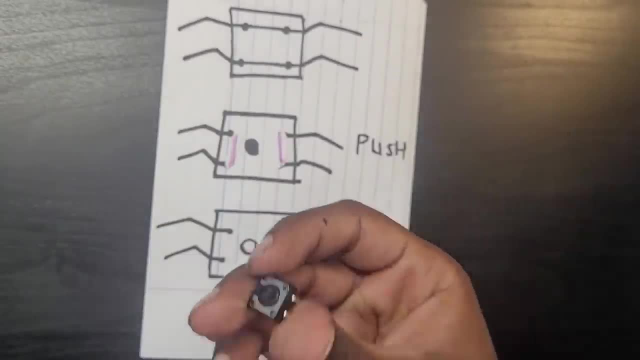 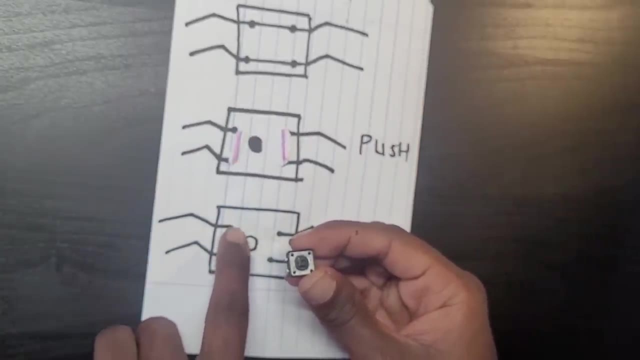 current, what flows? okay, basically, when you don't touch it anymore. by the way, when you just leave it like this, what's gonna happen? it's gonna be open. can you see this? so electricity cannot flow from here to here, but as soon as you push it down, what's gonna happen? as soon as you push it down, the wire is gonna go down. 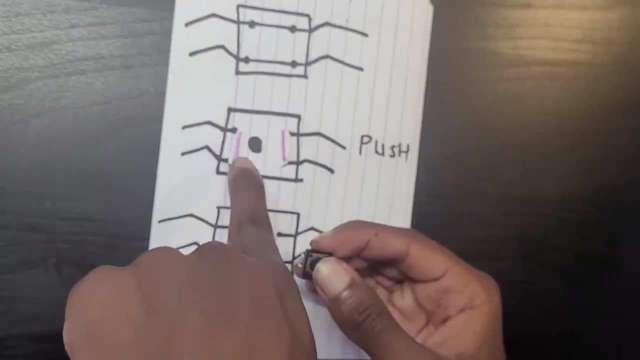 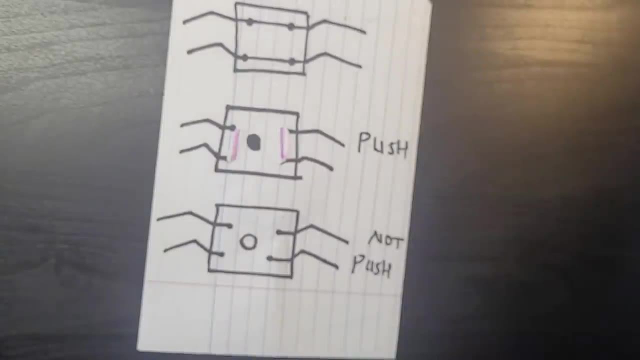 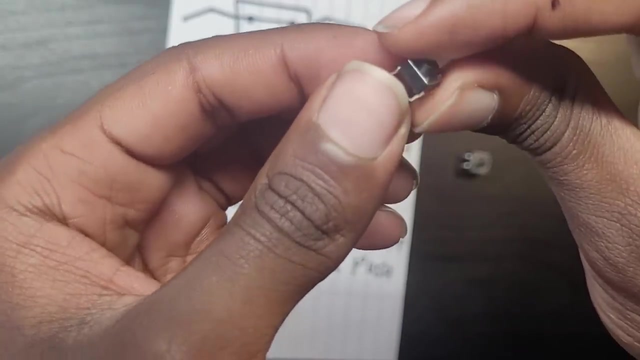 you're gonna push the wire down right here. basically, what? creating what? creating a complete circuit, in this case current- will flow. okay, so that's all you need to know to start with these. but one thing i want you to keep in mind is this: okay, when you look at the smaller, uh, push buttons, when you look at them, let's bring. 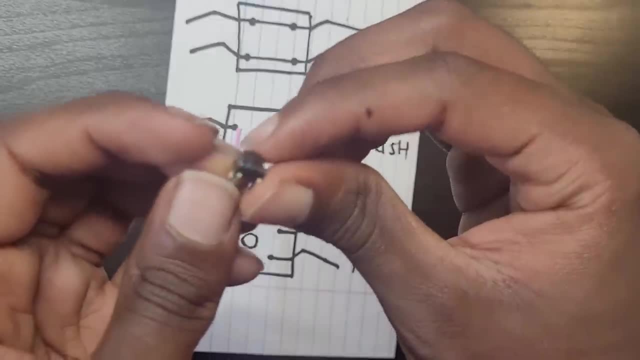 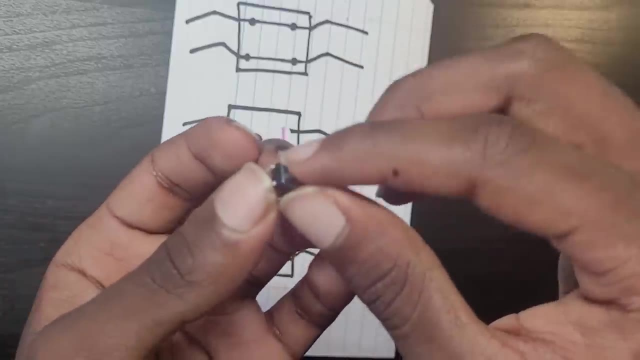 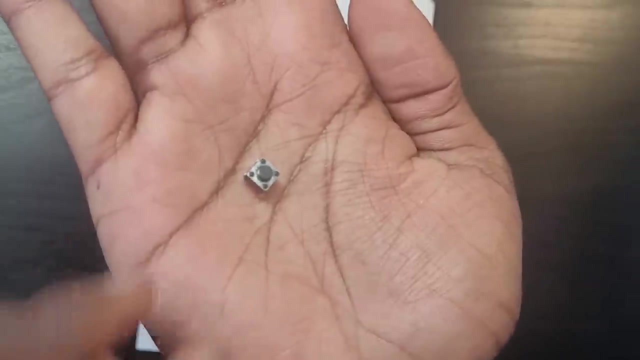 them here. when you look at them, it's really hard to distinguish. it's really hard to distinguish which side is which. am i supposed to put it like this? like in this way, let me just actually focus this way better. let me actually put it like this: it's better that way. all right, there we go, am i? 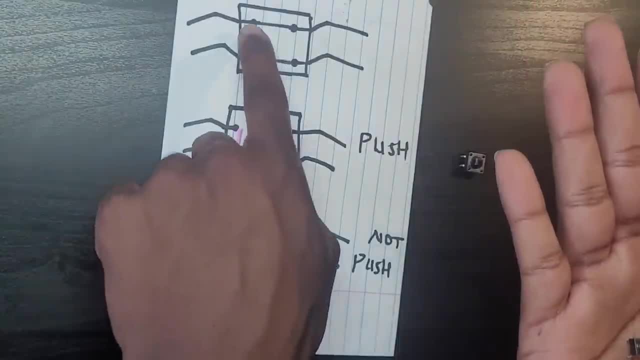 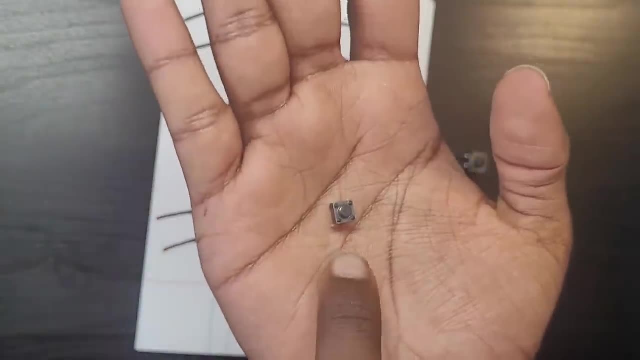 supposed to put this like this: you know how am i supposed to know which one is connected like this, which one have this type of connection and which one has this type of connection? because it's really hard, because they're symmetric. when you look at them, they're. 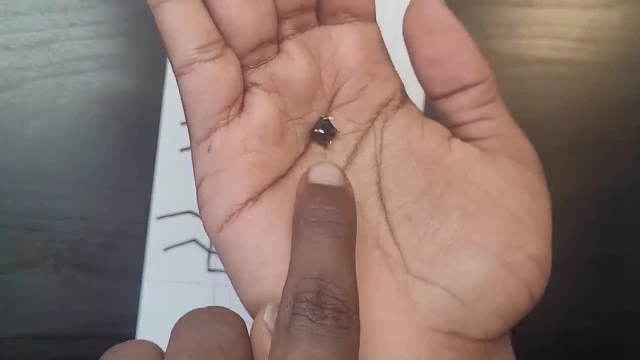 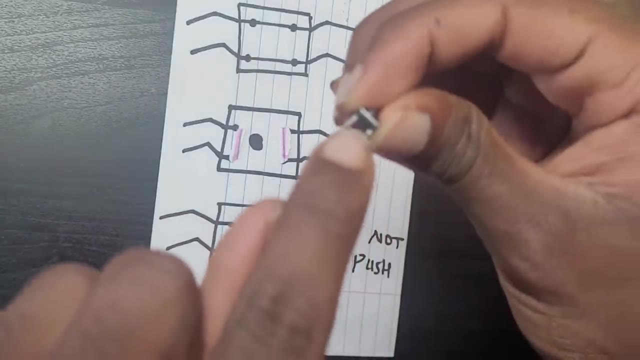 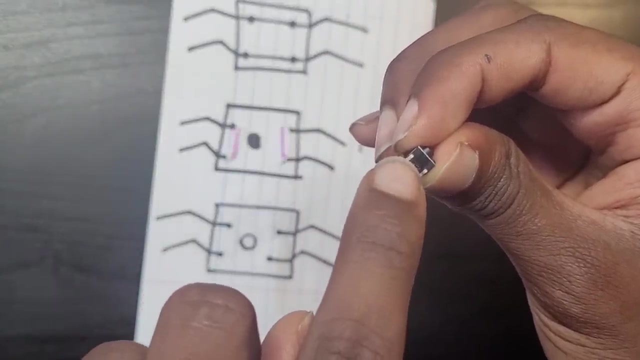 symmetric from both directions. they're at the very edge and you don't know which one's which. so always what you need to look for is what you need to look for: a side that have two pins. let me just focus right here. you always want to look for a side that has what? a side that has two pins. 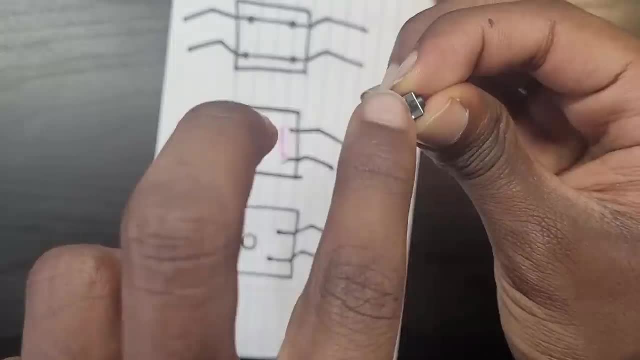 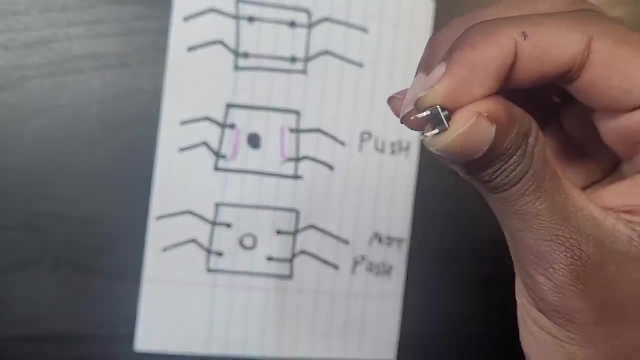 that are connected. so we're going to look at one single side here and they're what? they're connected to the same what, to the same side, right? so these two pins are connected to what- the same side. so you want to look at these. these ones are the ones that are where the switching is going to occur. i 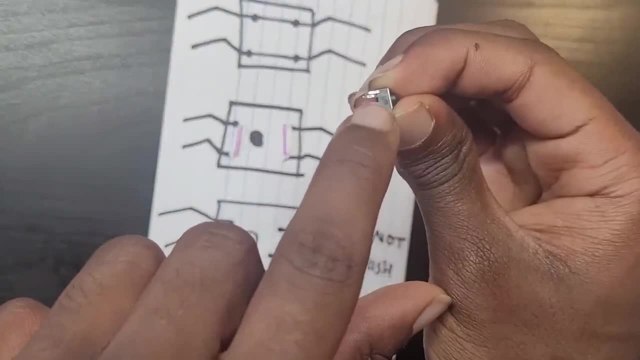 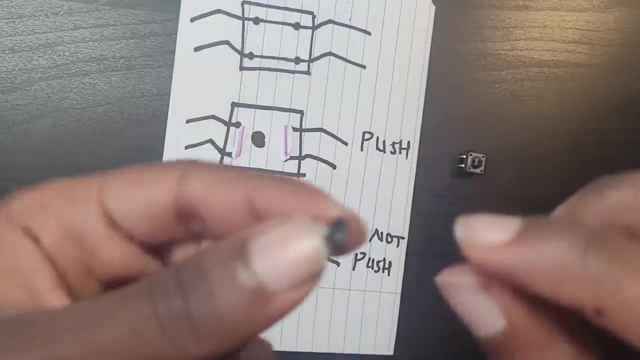 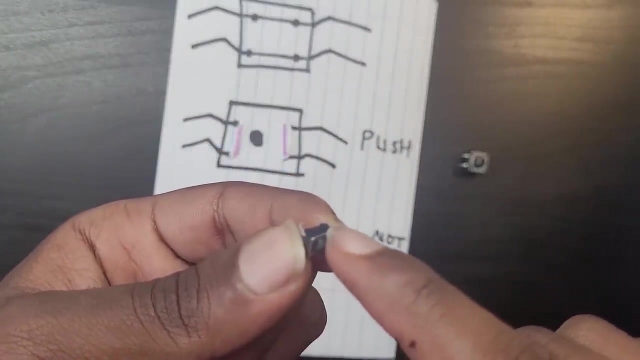 want you to keep that in mind. these sides are what, the ones where switching occurs. when you look at these side, when you compare this one with this one, we just bring it open here. wait, it's not focusing, my bad. okay, there we go. when we bring this one and this one, okay, these ones, they're. 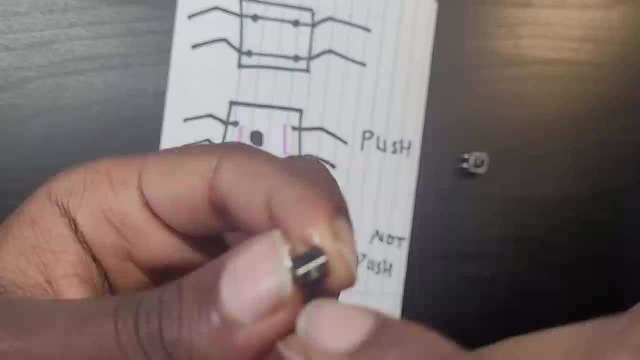 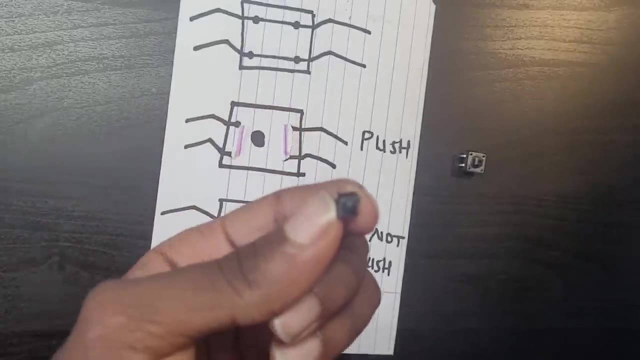 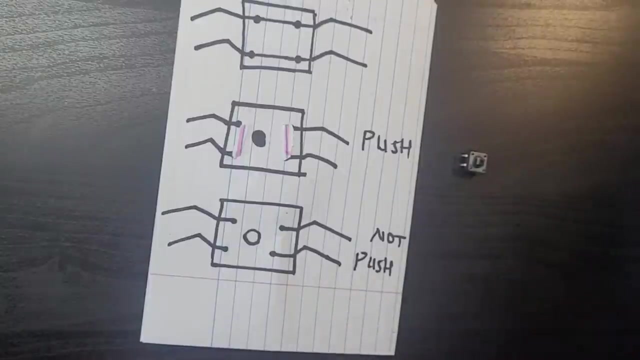 parallel. i want you to keep that in mind, because why they're opposite? they're not connected to the same side. okay, so the ones that are not connected the same side. what happens to the ones that are not connected to the same side? the focus is really bad. oh, my, it's really bad. focus, right? what happens? 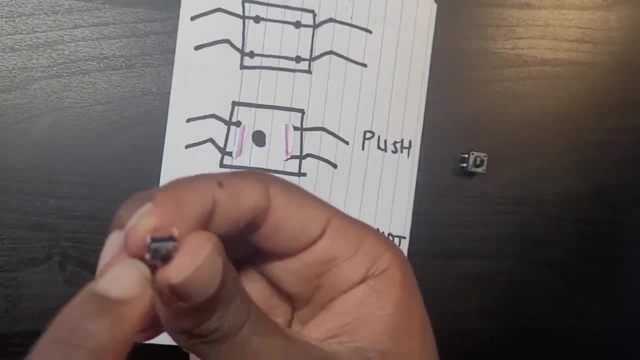 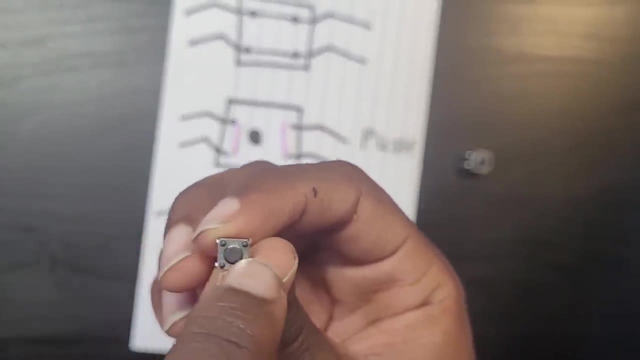 to the ones that have um, that are connected to the opposite side. okay, i want you to look at the parallel sides. so this side is right here, there's a parallel side right here, so the ones that are connected to parallel sites are connected in this way. they're always connected. okay, either you push up or push down, they're always connected. 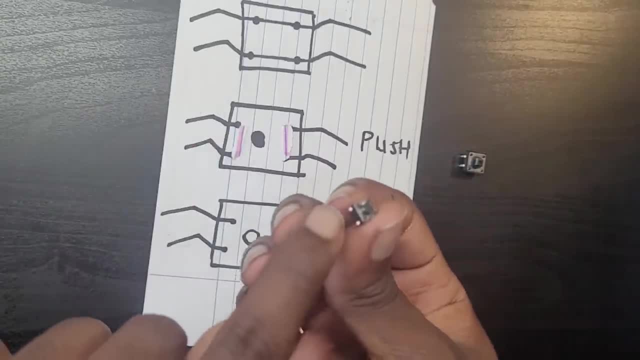 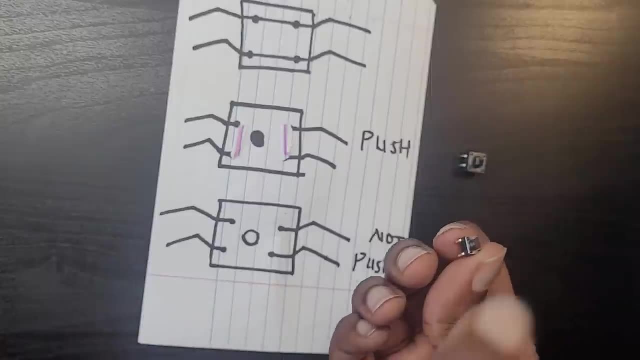 okay, so. so when it comes to the ones that are attached to the same side, what is what happens? they're connected and the and the metaphor is connected in a condition: if you push the button, it's connected. if you don't push the button, it's not connected. 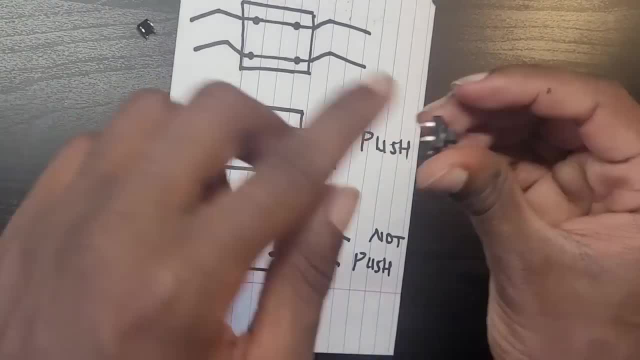 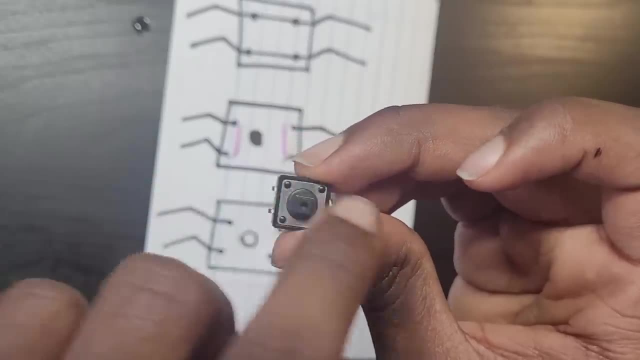 the ones that are facing the same side. okay, the same goes for this one too. so i want you guys to again to use the side metaphor instead of, uh, using the ones that are far apart, because in this one, everything is. when you look at the small one. i'm just playing the small switch. 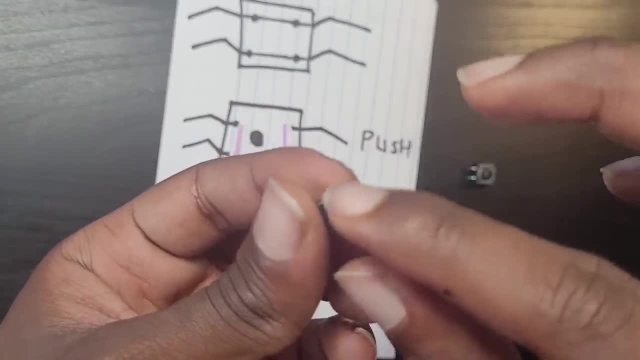 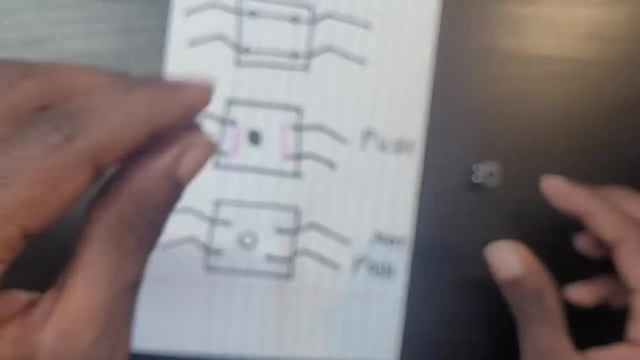 when it comes to a small switch. everything is what, everything is equally distant. okay, it's a square side, it has a square shape, so everything is going to be what equivalently distant. so again, look at this side. so the ones that are connected to what, the ones that are on the same side, 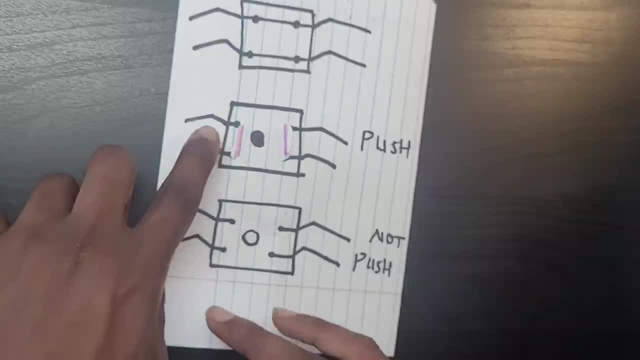 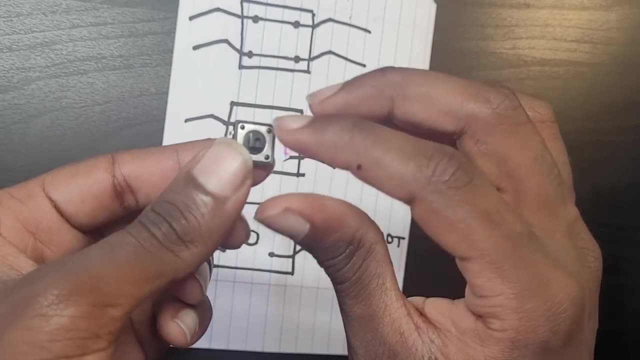 the same pit, the pins that are on the same side have what they're going to be: the ones where switching is going to occur, the ones that are connected parachutely on the opposite side. basically, the parallel sides are going to be what are going to be: the ones that are always connected. 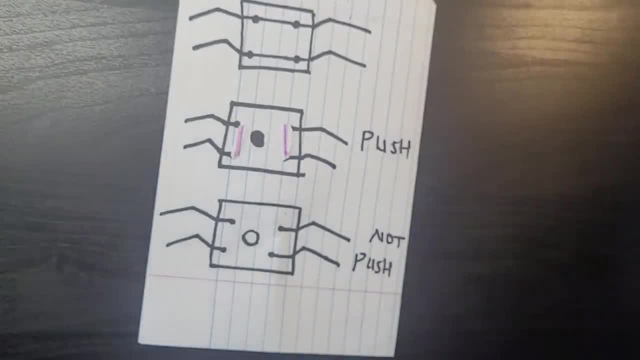 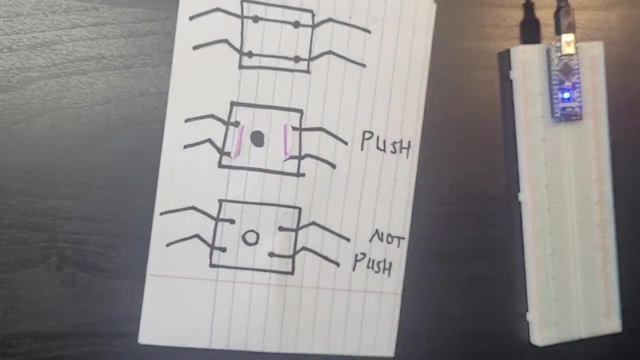 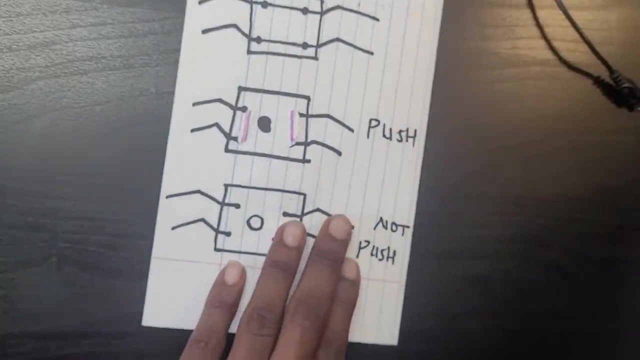 either you push up or push down, they're always connected. i think it's going to make more sense when i just bring my arduino right here, okay. so let me just bring this right here, okay, and let me just unplug my arduino for now. let's just put this to the side so that you guys could. 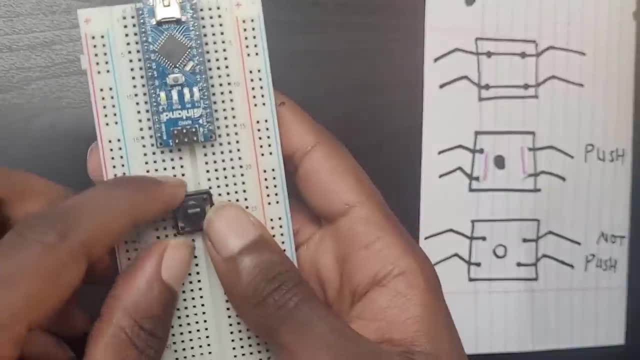 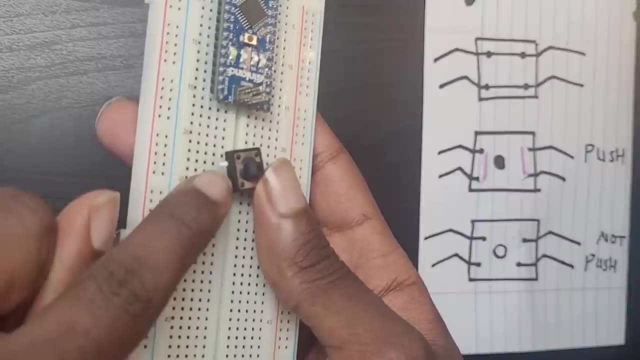 actually reference it. let's put this to the very edge, okay. so let me bring my arduino right here. how am i supposed to connect this? i'm supposed to connect the ones that have the same side- again, the pins that are on the same side. okay, the pins that are on the same side. how do i want to connect? 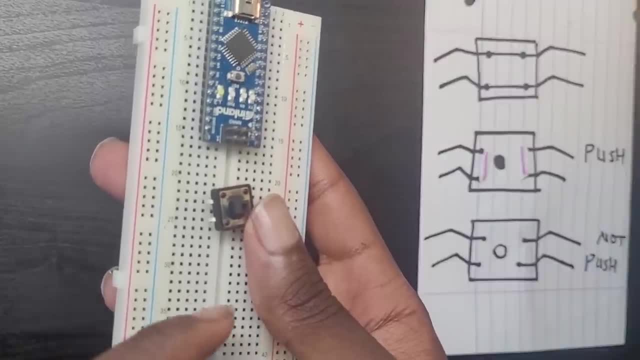 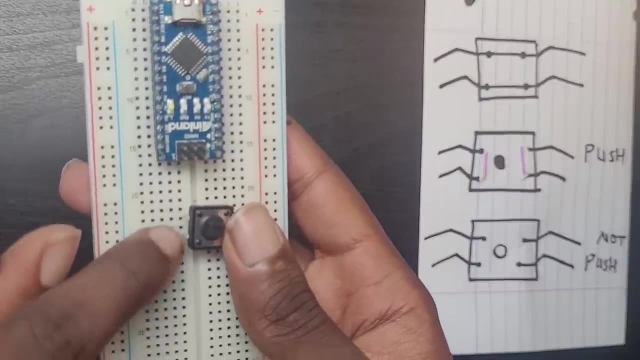 them. i want to connect them across. i don't want them to be together. if that was, if they are together, obviously what switching cannot occur. so i want them to be in what opposite? what in opposite? obviously in opposite rows, right here. i want them to be in different rows, okay, so i'm just 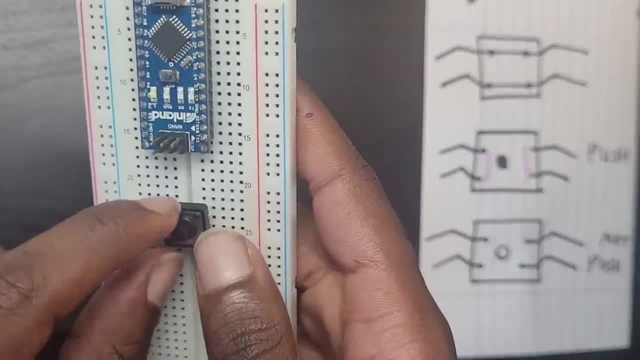 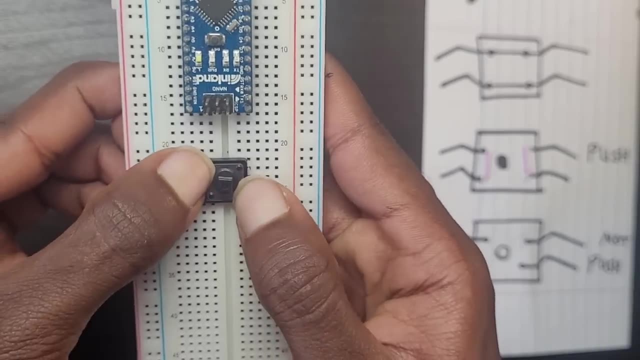 gonna push it in as much as i can. i'm gonna put this across too, okay, because it makes more sense, uh, to put it across, i'm just gonna try to. all right, there we go, at least a bit of a push. all right, there we go. now it's uh, now it's plugged. 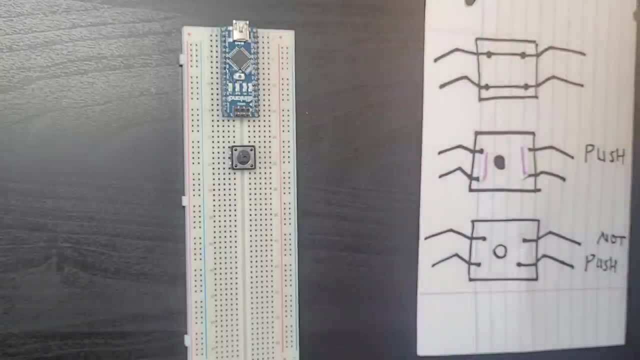 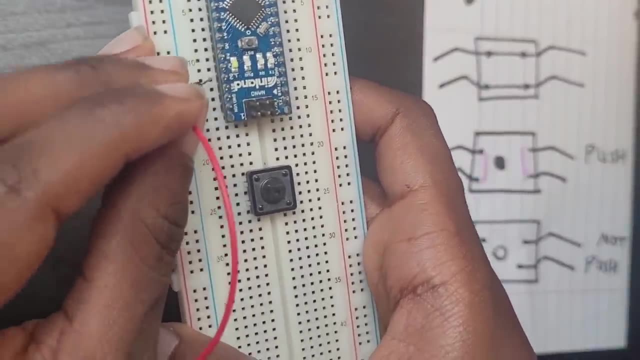 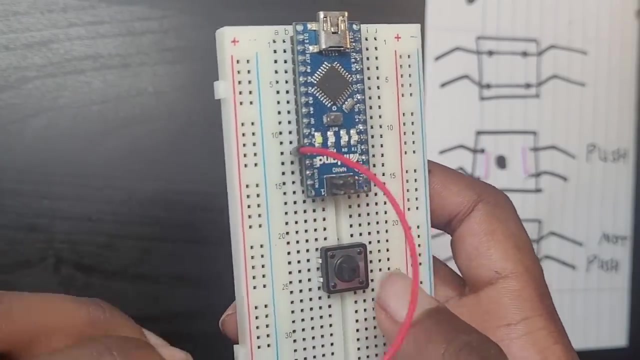 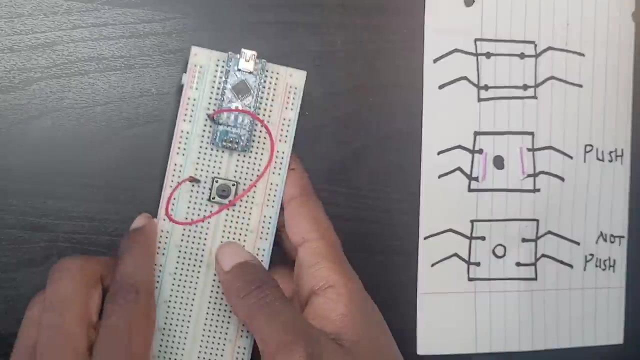 in all right. so right here, let me just bring my my red pin and connect it to a five volt. what i'm going to do is build a simple led circuit, but in this time, what's going to happen? i'm going to be on the first, but on the first one, on the first leg did that. now i'm going to need a resistor. 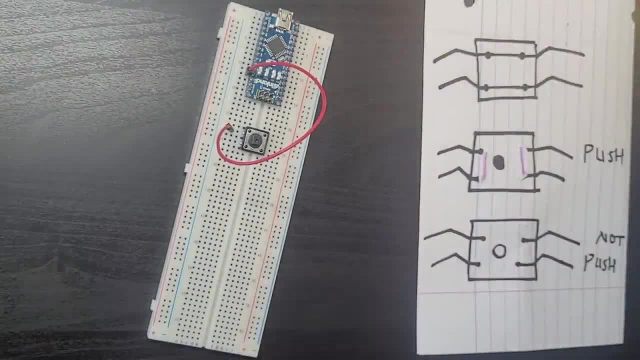 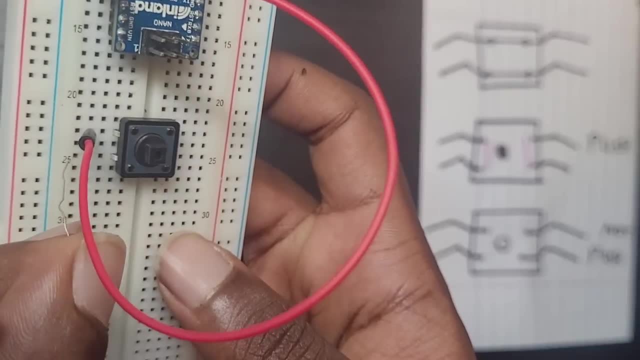 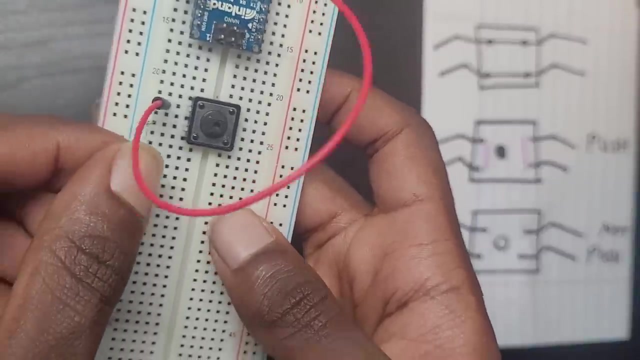 where am i going to connect the resistor? because i want switching to occur. i'm going to connect it to the what? to the second leg right here. second legs right here. i'll have to disconnect it. let's do that right here. okay, there we go. second leg is connected, the resistor, and then i have my. 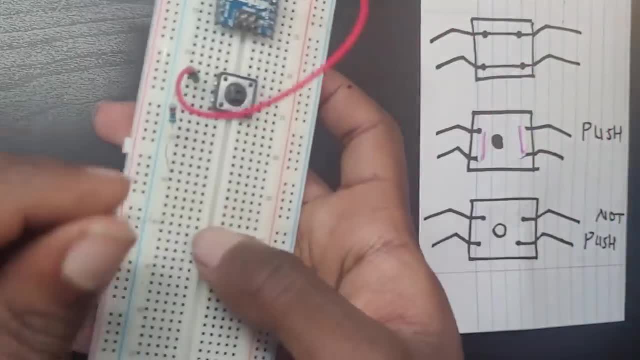 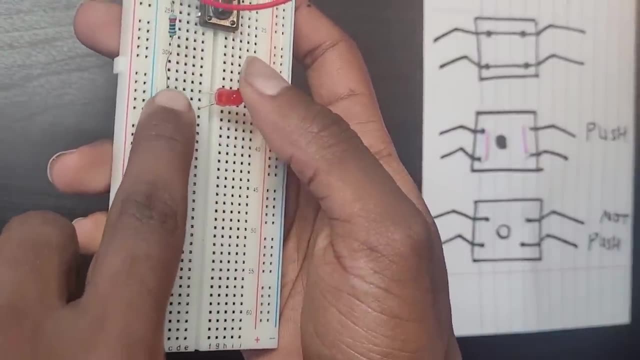 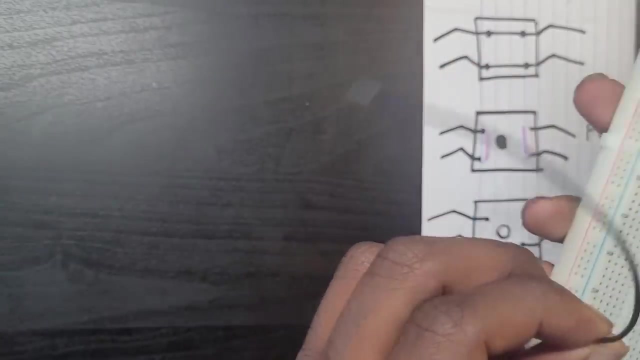 obviously led light. let me just bring that, just bring my led light. there we go. led light is connected right here to the what, to the leg of resistor. right here, you can see it. and then obviously i'm going to need my gnd, my what, my ground pin. let me just get it right here and 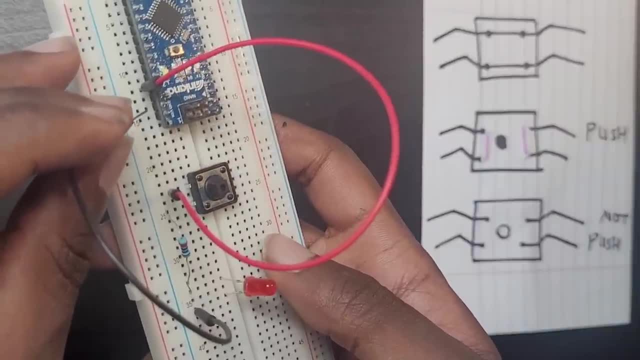 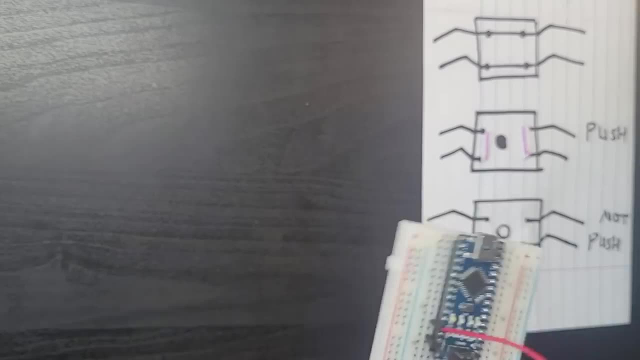 connect the gnd. let me just make sure that i'm connected to the gnd. i don't want to get it wrong there. we go to the gnd, okay, so now what i'll have to do is what plug in my arduino? let me just do that. 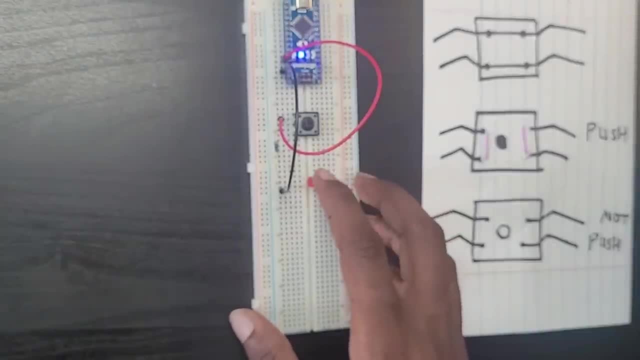 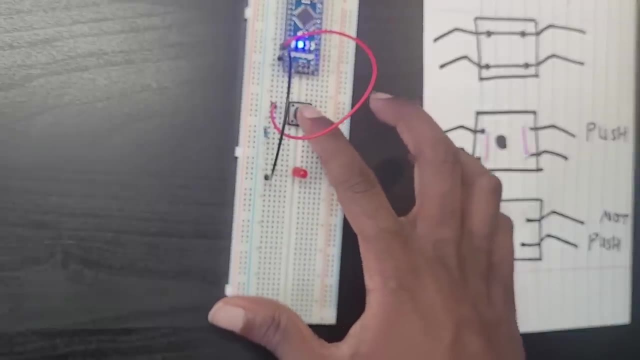 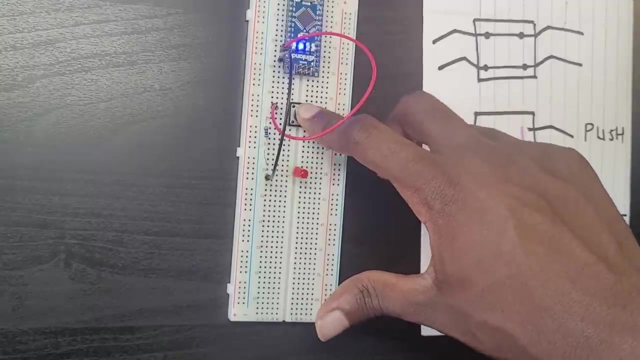 all right seems to be working. okay, the arduino is on. uh, let me check my resistor, if it's okay. okay, let me just push on the button right now and let's see if it's going to turn on or off. okay, there we go. it's turning on, as you can see, it's turning on, but as soon as i let go, look what. 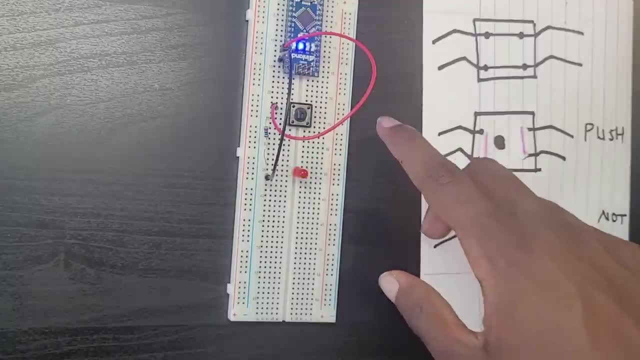 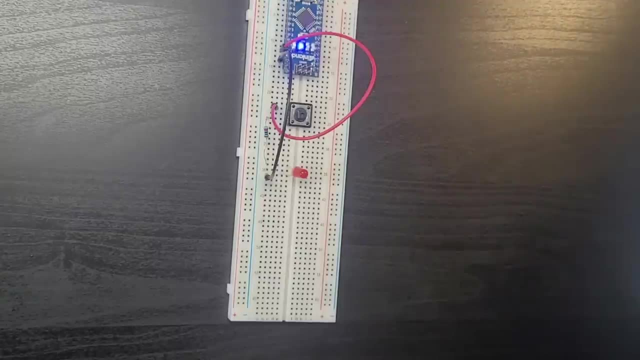 happens. i just i just touched the button and it's going to turn on. and it's going to turn off to one. let me just touch it once. as soon as i let go, it turns off. so one thing you need to understand here is these buttons that i have right now. they're called: where's my sharpie? right here? 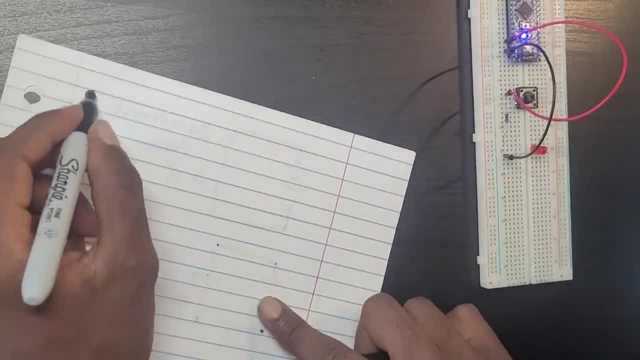 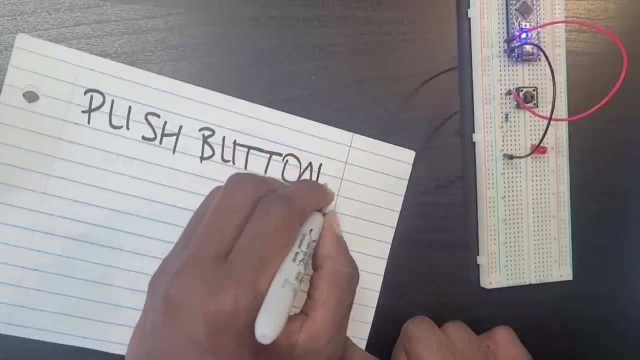 there we go. there's my sharpie right. they're called push buttons. push buttons, okay, push switches. basically they're switches. that what they're? push buttons or switches. how about the one that we use most of the time for a lot of insurance? l protected computers or something like that, right? 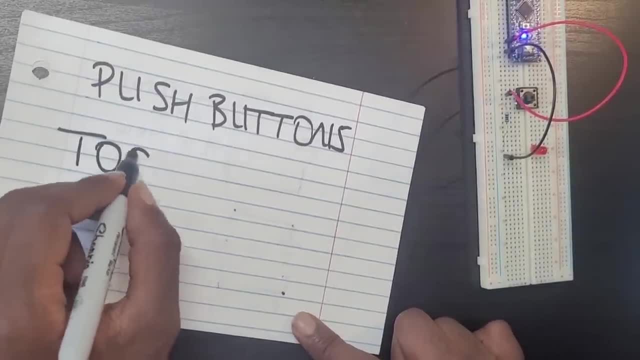 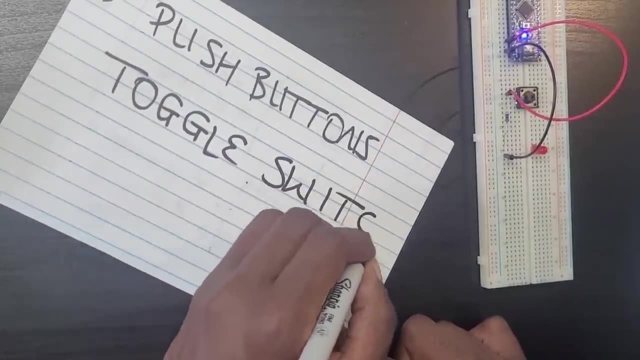 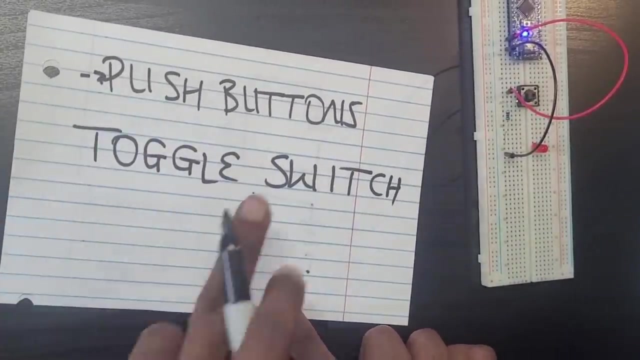 so anyway, let me just touch it once. let me just touch it once. as soon as i let go, it turns off. so one thing тор mostly we use is called a toggle toggle switch. okay, so right here, when it comes to push buttons, the name gives you a push button, i just want you. 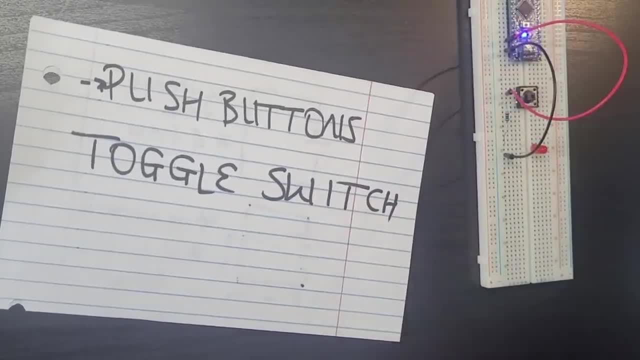 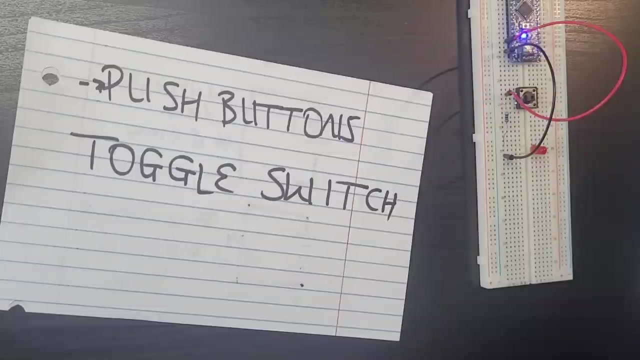 to think of it as a push door. okay, as soon as you let go of a push door, what happens? it goes back to what? to its original position. okay, as soon as you let go. all right, when it comes towards um, the doors we have at home and stuff, if you don't again put excess amount of 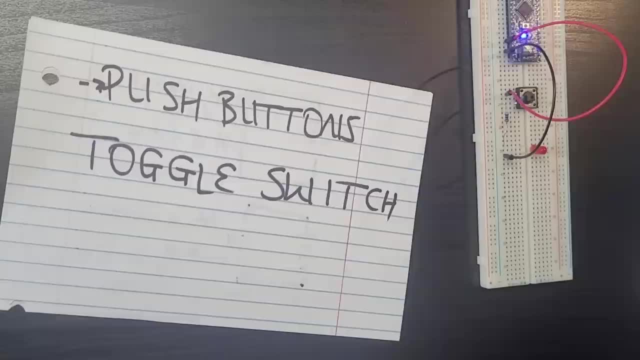 force. what happens is, if you just put it in the middle, it's going to stay in the middle. if you just leave it there, if you just again push it and then you leave it at a position, it's going to stay there. it's not going to move enough itself. it's not going to what close by itself. 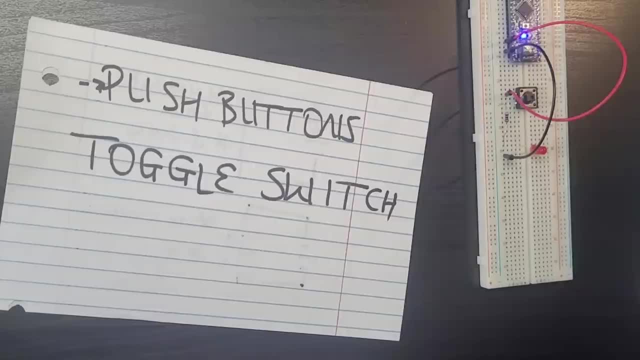 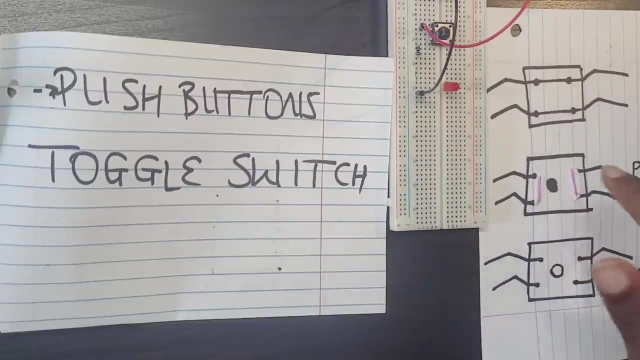 just like how again push. uh, push doors do okay. so i want you to keep that in mind. when it comes to push buttons, you always have to push okay for it to what for it to. right here, let me bring my paper for it to always- what for it to always connect you always. 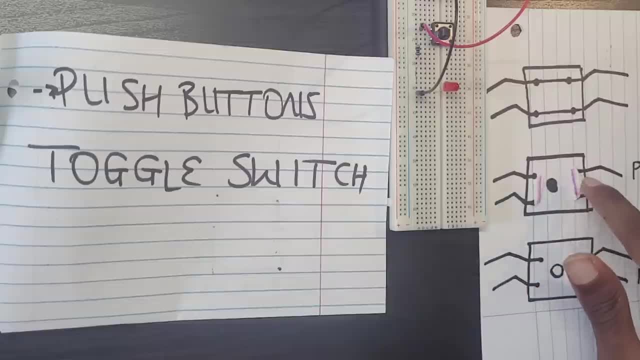 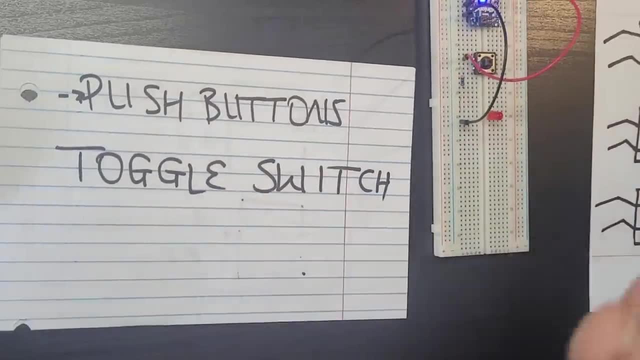 have to push to what? for it to always put down this wire right here, okay, this connecting wire right here, so that what it switches switches on. okay, so you always have to push when it comes to toggle switches, the ones that we have at home. what you have to do is what you only touch it once and 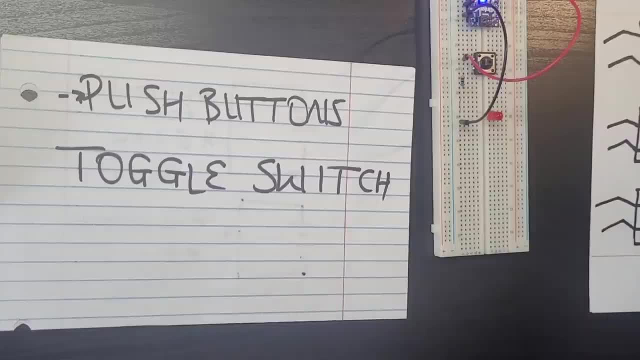 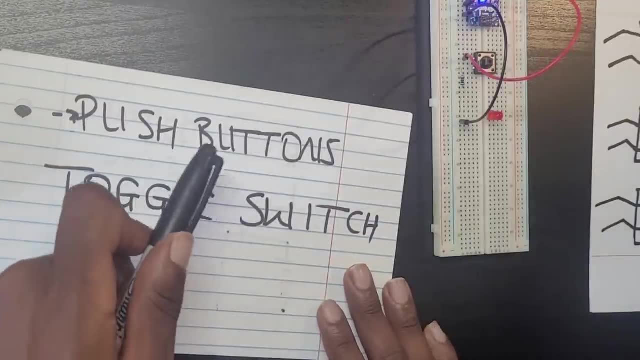 you turn it on. that's it. that's all you need to do. but again, touch it again and what's gonna turn off will turn off when you let it go. so now you have to make sure that this is connected, okay, so i'm going to turn off the switch or the button. so right here we're going to be using push switches. 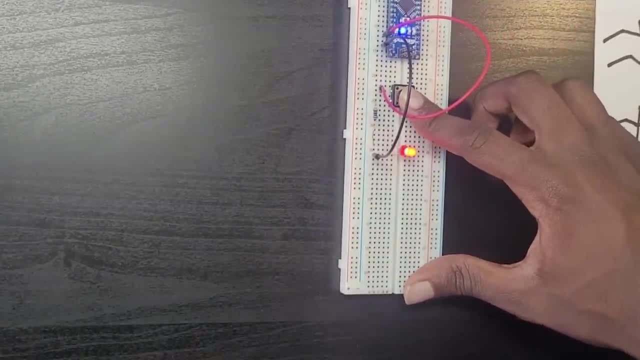 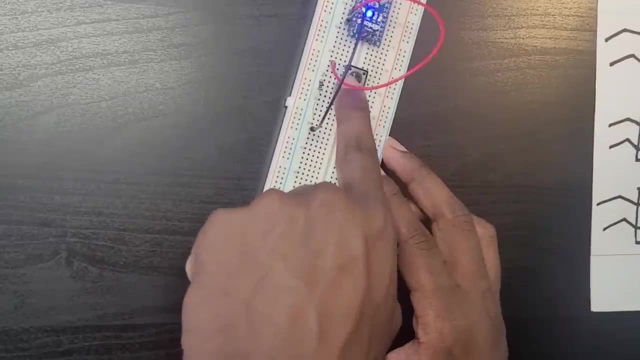 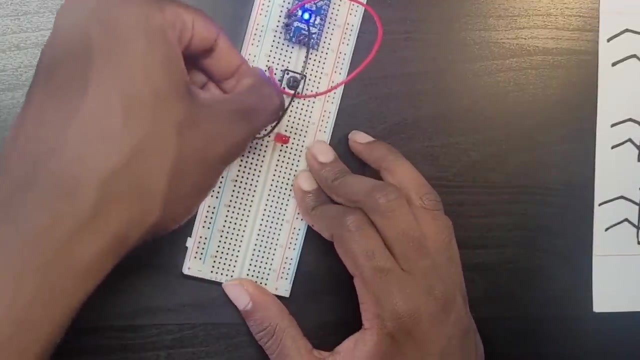 or push buttons here. okay, so we have push buttons. so as long as soon as you let go of, again, as soon as you let go of the switch or the button, what happens? it turns off. okay, there we go. so let me just bring this here and let me try to connect it to the one that is parallel right here. let me just 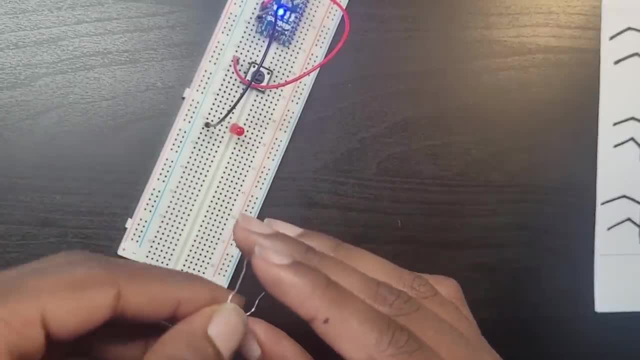 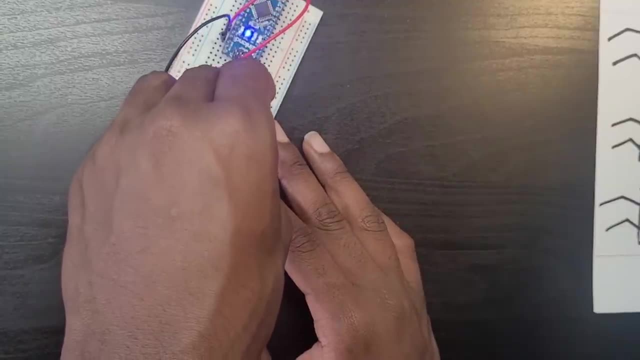 try to do that. so i'm giving my resistor right here. just pull it out. you've seen that it works. the what when we're using the pins that are on the one, the legs that are on the same side. let me just try to connect and try to connect the ones that are parallel. okay, let me just do that again. let me. 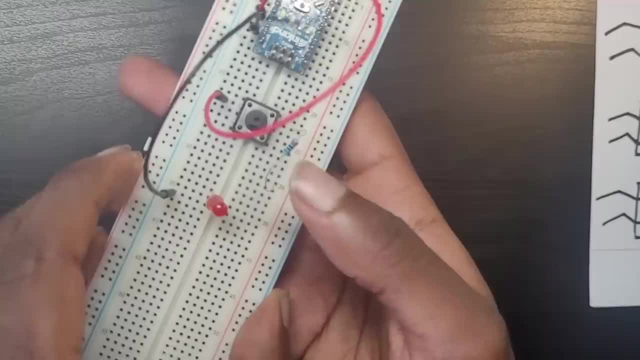 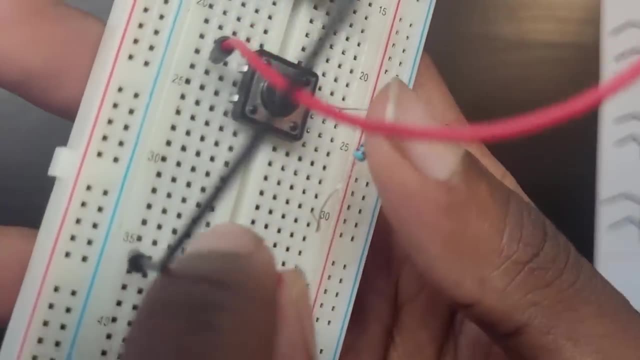 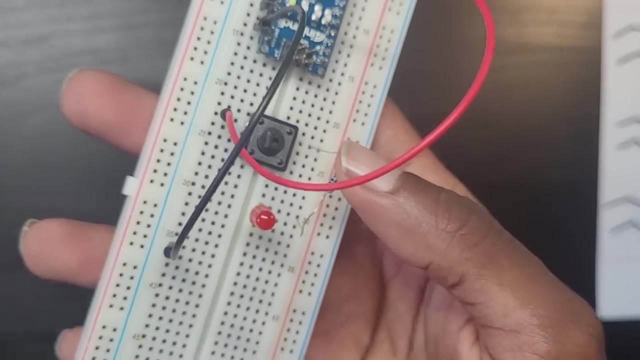 just unplug my arduino because, again, it's better to what to always unplug your arduino work on your again physical project and then plug it back in. okay, let me just do that. let me connect my led to the leg of the resistor- okay, and i need to connect my what, my gnd? okay, everything seems to. 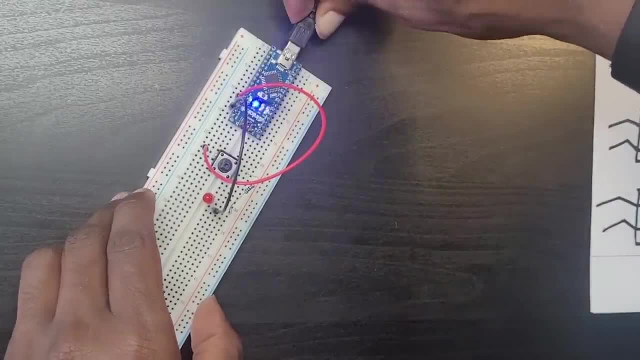 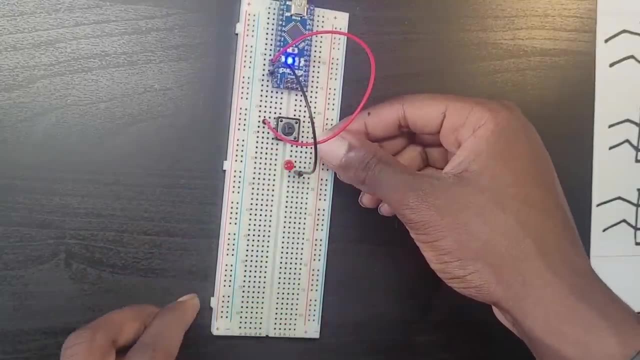 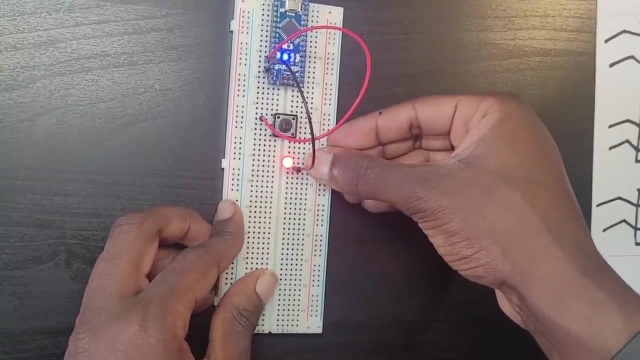 be good and everything should be running by now. let me plug it. okay, my resistance is the one that is causing the problem. let me just go here, push it. okay, this leg is not pushed. let me just push it. let's push it really hard. okay, i have to push it really hard. 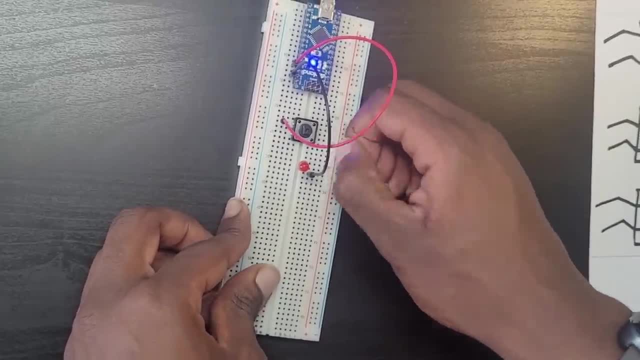 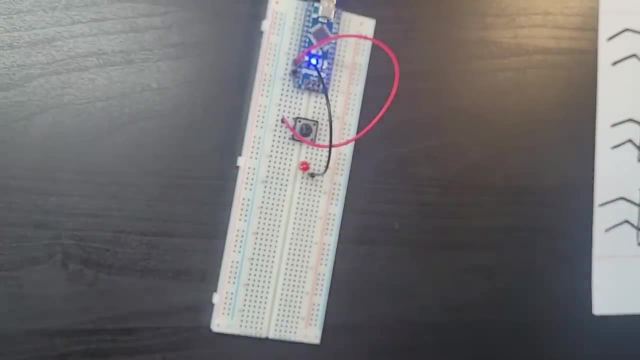 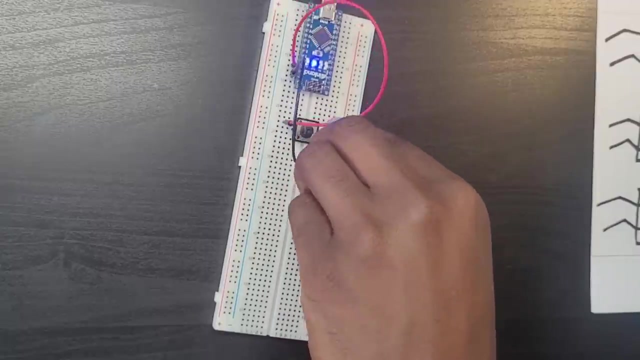 okay, wait, let me just get my resistor. let me let me fix my resistor right here. i think it's the resistor that's causing the problem. i think it is. as soon as i push it back in, it's gonna work. let me just go over here, push my resistor. jesus keeps bending, the leg keeps bending. 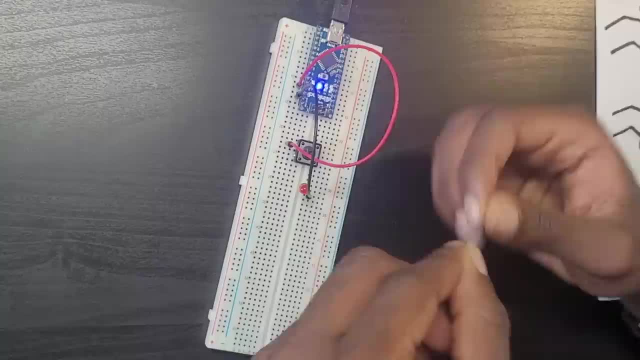 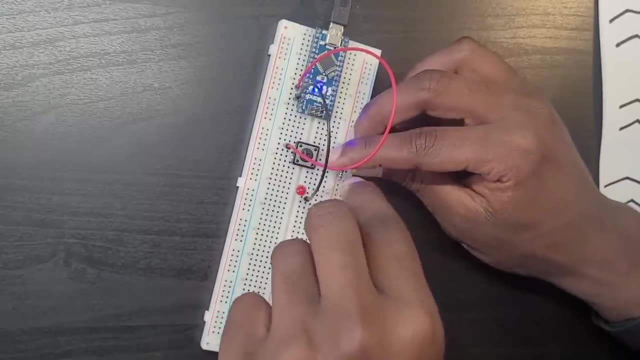 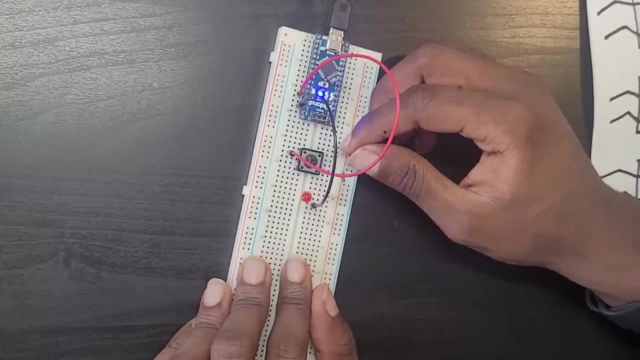 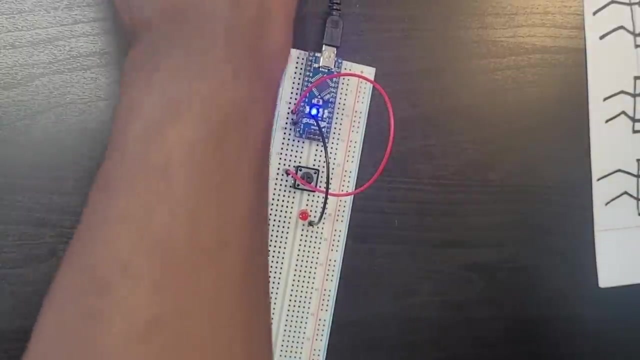 wait, i need to straighten this out first. let me straighten it out, all right. all right, connect it right here, come on. is the resistor connected properly? oh yeah, i think it is, but okay, the resistor is a bit coiled. i'm gonna have to fix this. let me just 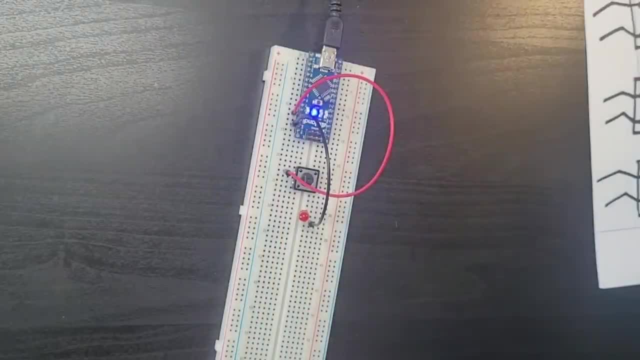 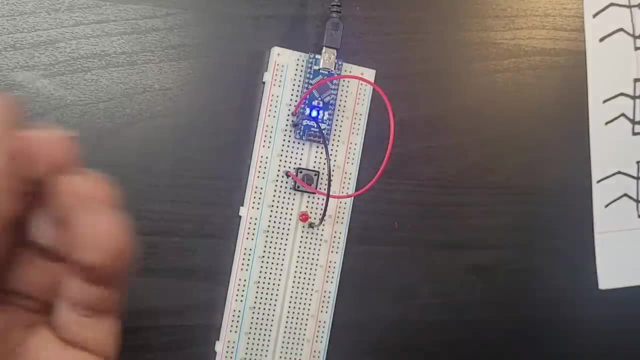 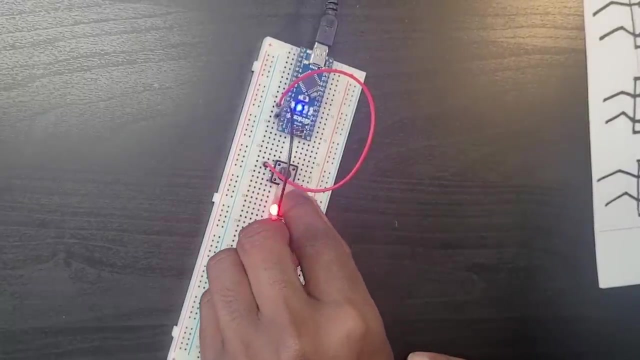 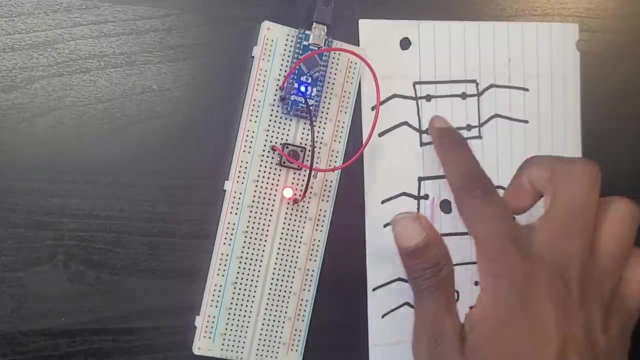 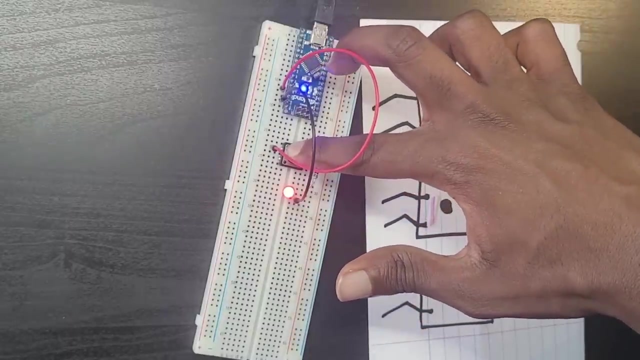 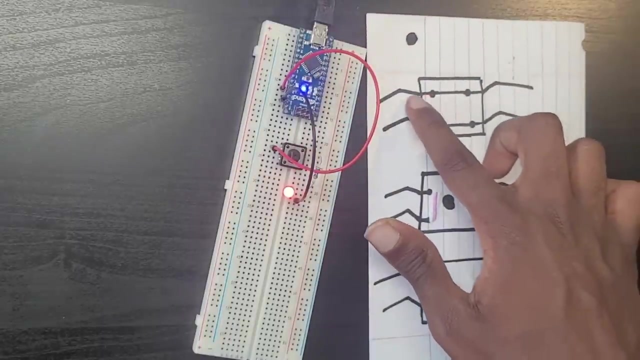 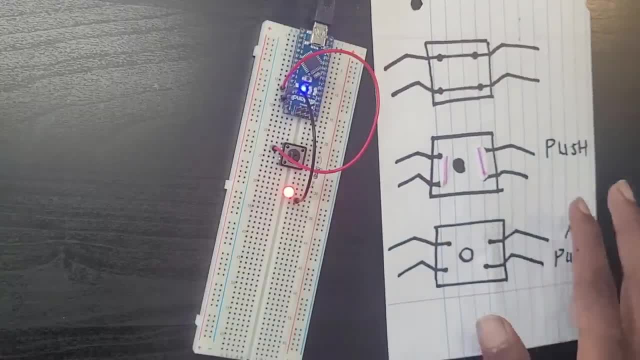 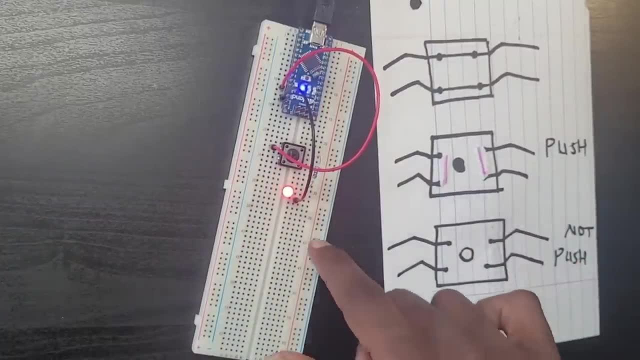 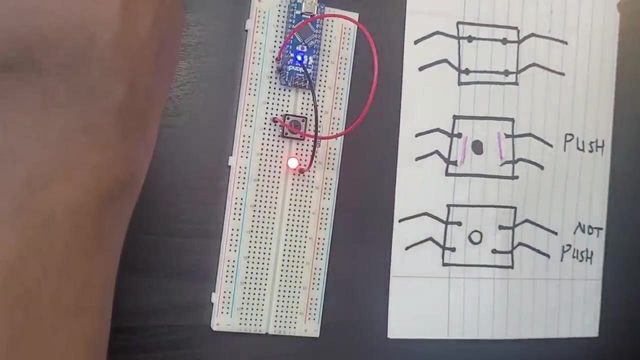 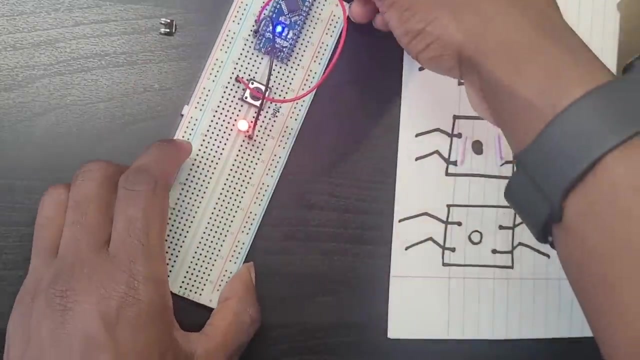 regardless of them being pushed or not. okay, but when it comes to the again, the ones that are on the same side, what happens is again, again, we have to push to what to basically connect them. so this is where the switching occurs. all right, let's just do this. um, using the smaller pin right here, let me just do a smaller one. i have not used that. but before doing that, actually, i have a really, really a good question. okay, let me just unplug this right now. what i want you to do is i'm going to put this: 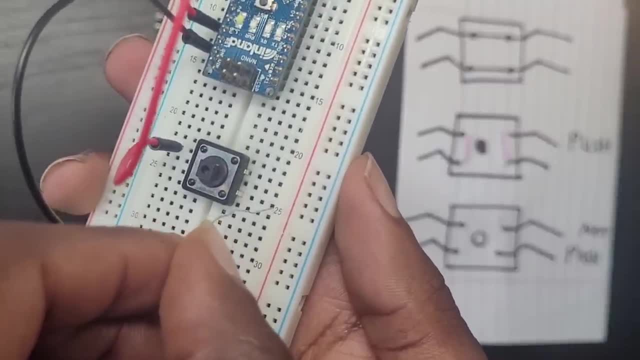 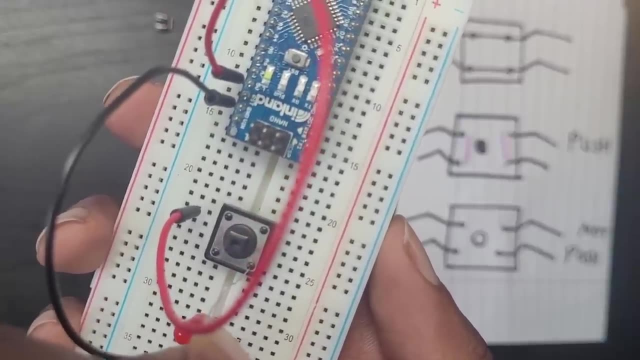 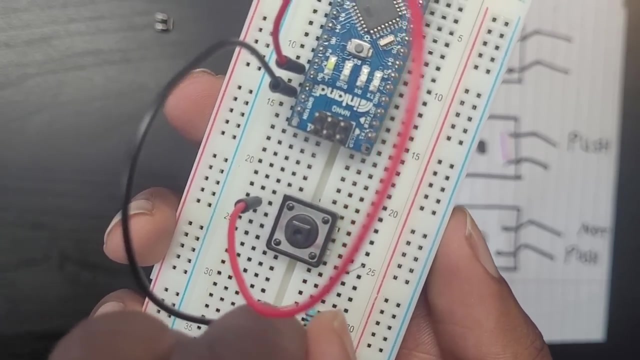 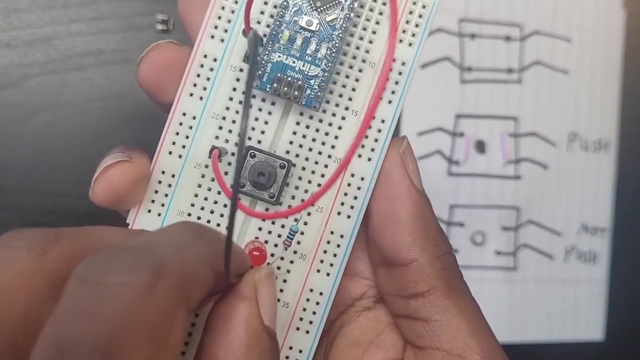 all right, as you can see, i'm going to put this, this, at this third leg. right now, they're not parallel, they're more of diagonal. i'm just going to put this one connected to this. okay, i'm going to be connecting it to what? to this one, the one that is right here, to the leg that is right here. what do you suppose is going to happen? let me just go right here. what do you suppose is going to happen right here? i mean, i'm connecting this one to what to this. connect the first one to this one. they're more of diagonal. 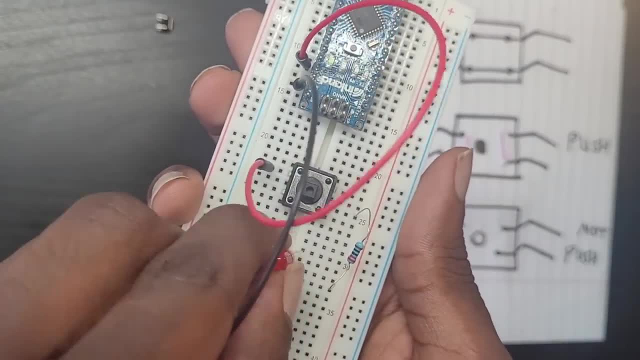 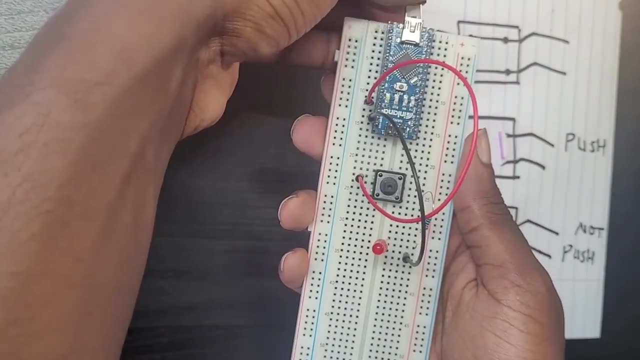 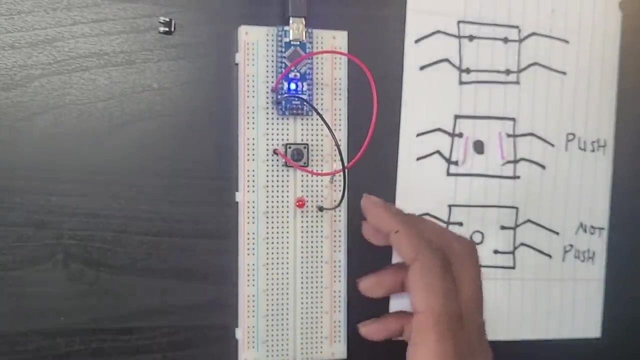 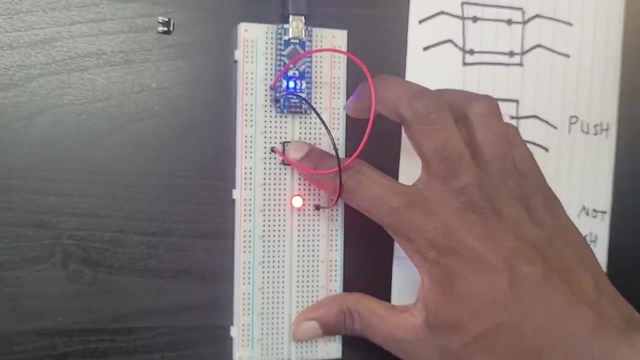 diagonal. all right, let me. i have to adjust my arduino again because i touched the resistor. there we go. the gnd is back here. let's see what happens. what do you think is going to happen, though? it's the real question. okay, so i'm just connecting my arduino, so let me just show you what happens right now. you might be wondering why is this working as a swift? we just said that. you know, the ones that are on the same side are the only ones that work as a 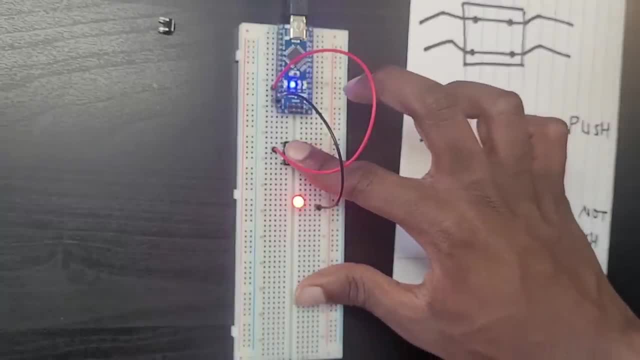 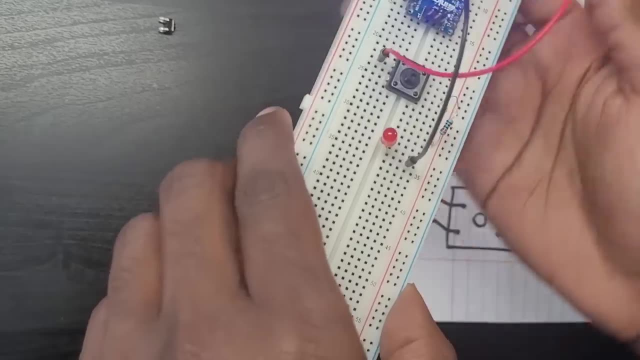 where the switching occurs. so you might be wondering what is going on. well, the simple answer is: what? as i said again, these the first one and the second one. let me just again bring my Arduino closer, right here so that i can explain it. let me point at it using maybe a pen, okay. 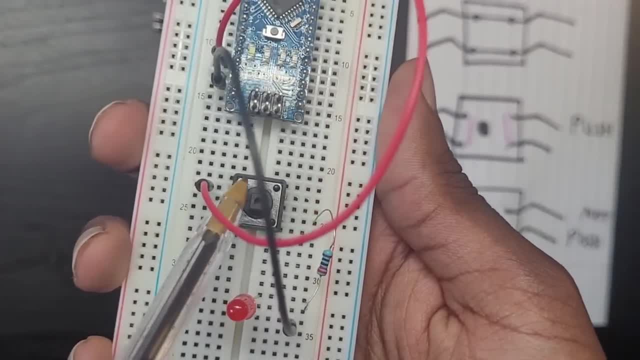 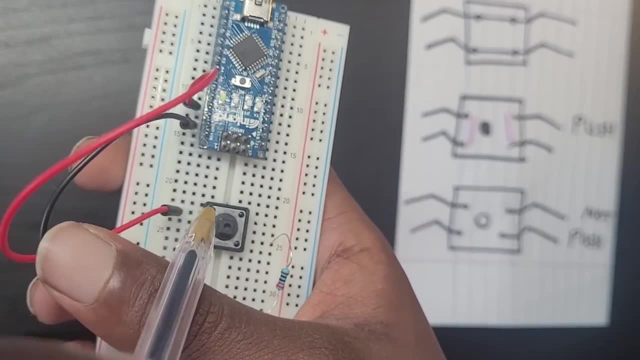 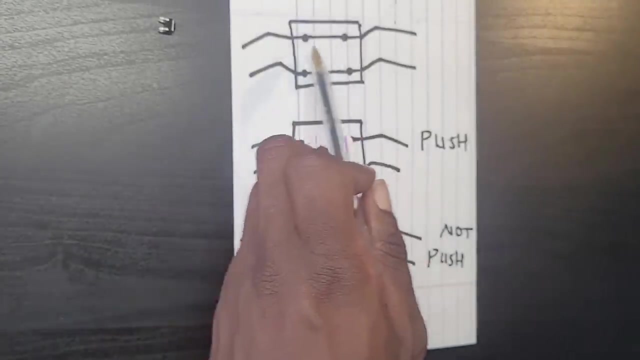 these Arduinos are what these sides are connected, as we said again. the first, let me just bring my, just take out the wire for now, let me just push it right here. the first two are always connected. as i said again, the first two are always what they're, always connected. they said again: they're. 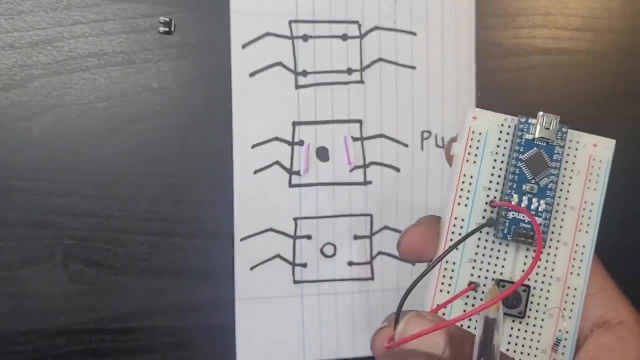 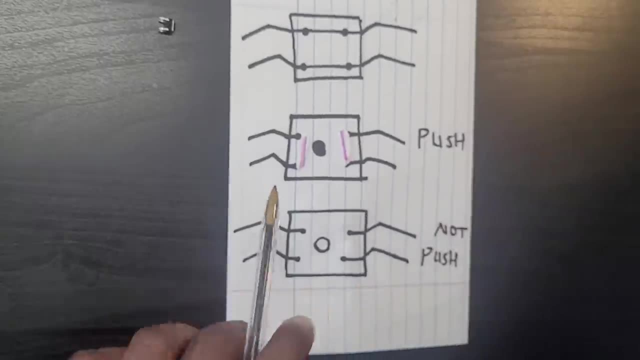 always what they're always connected. all right, so they're always connected. so this side is always connected to this side. so this side and this side is going to be what directly connected. and what did i say? this side and this side, basically, this side and this side, this side. 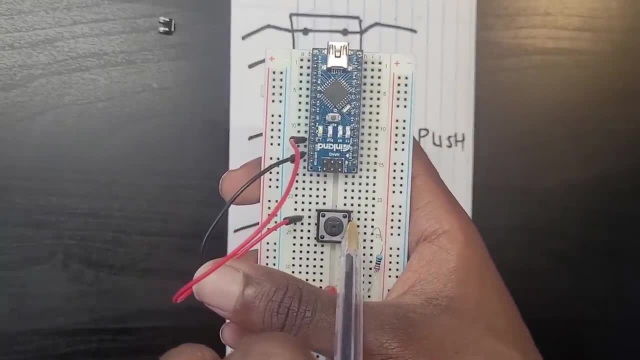 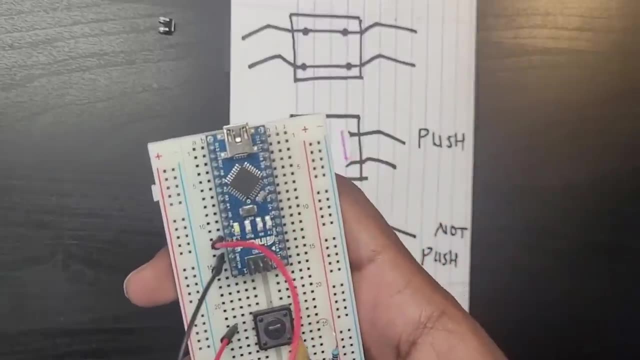 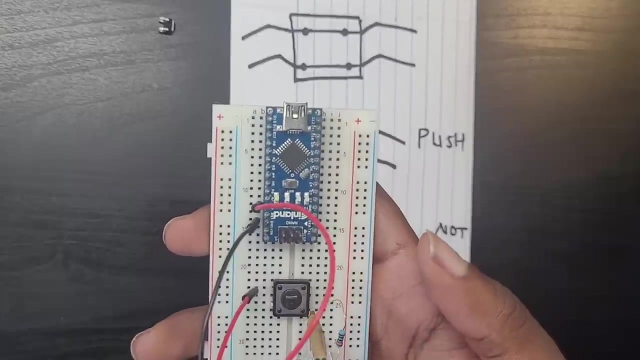 and this side, basically this and this, the ones that are, that are on the same side, are what. they're connected, if you want, if you push down again, again, this is where the switching occurs. so they're connected when you push down. so what happens here? this is always directly connected and then, when you push down, this also becomes. 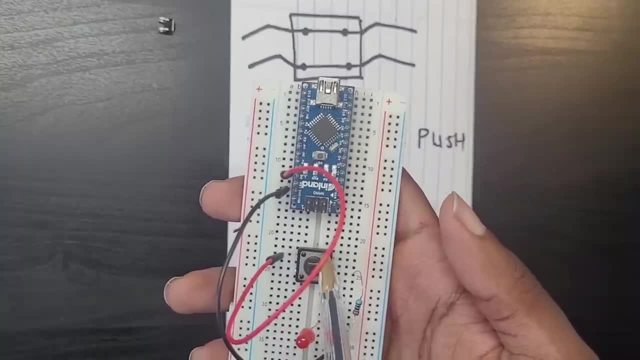 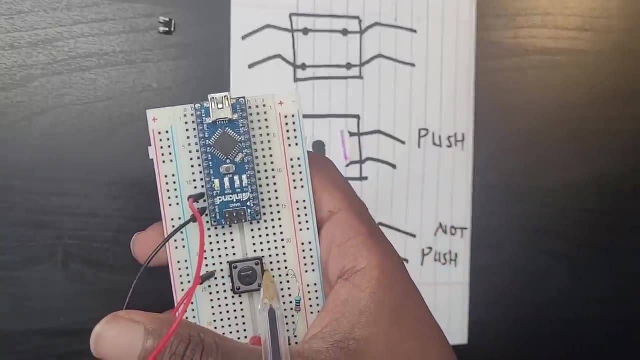 connected so you see, moves the electricity moves from here to here, which is always connected. just again, pull the wires right here, it's always connected from here to here. and then what happens? and then when you switch down this and this is connected so indirectly, what happens? this and 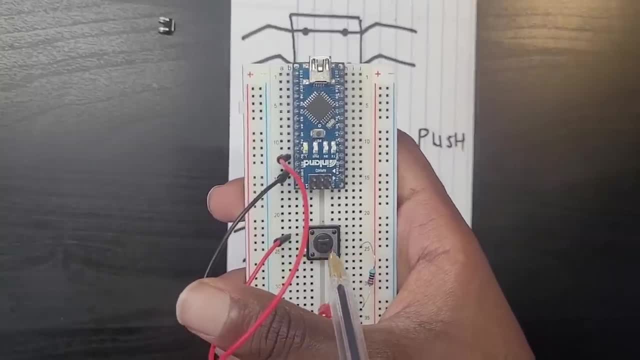 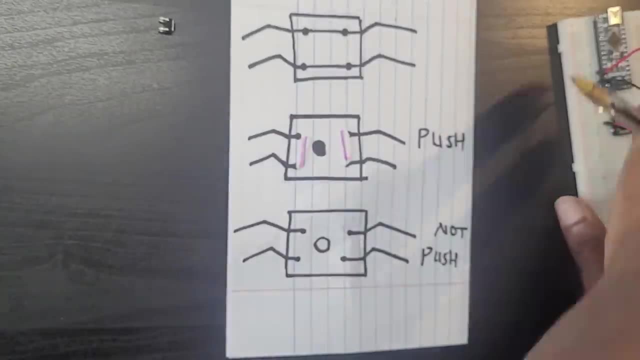 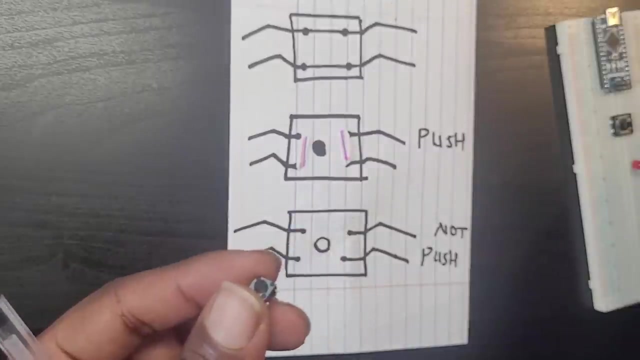 the resistor, the five volt, the red wire. again, this and this become what indirectly connected. so again, i just want you to keep that in mind, all right. so one final thing is before moving on um on this section is: this is a bit confusing for people. again, as i said, i don't want them to be confused, so let me just unplug everything. 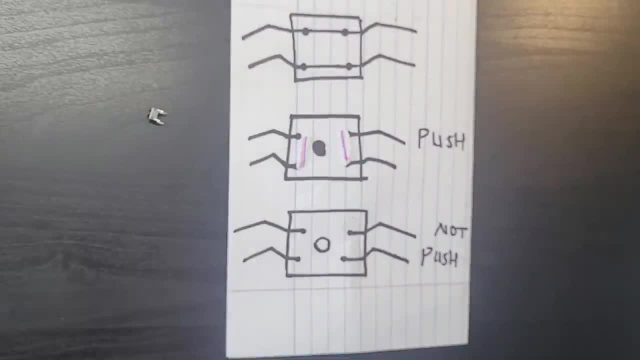 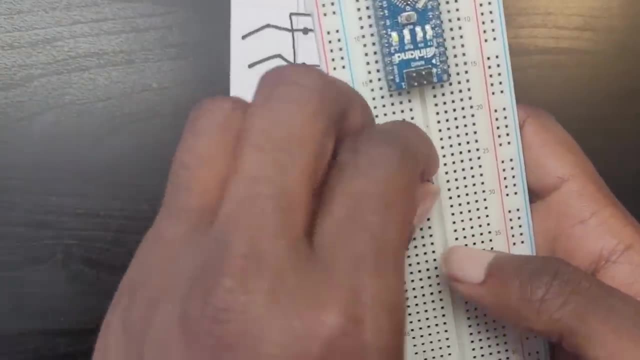 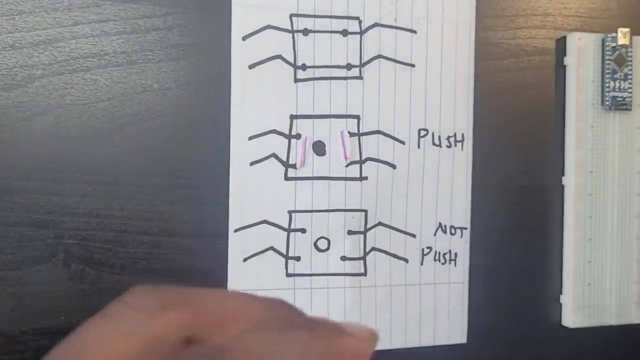 which is really hard to get off. all right, there we go. took me a while, okay, it's a bit confusing for people and i even had to do a lot of research before even making this course because it's a bit confusing, okay. so one thing again, as i said, is what we're gonna always look for- sides, okay, so 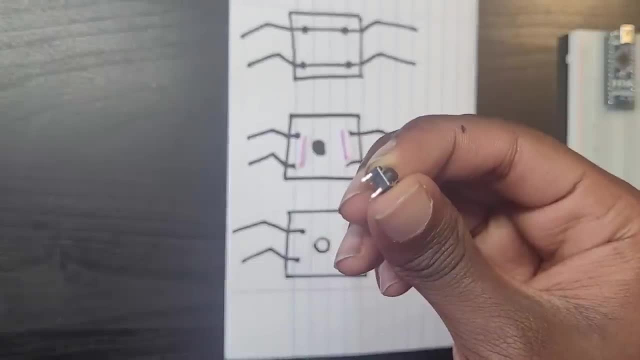 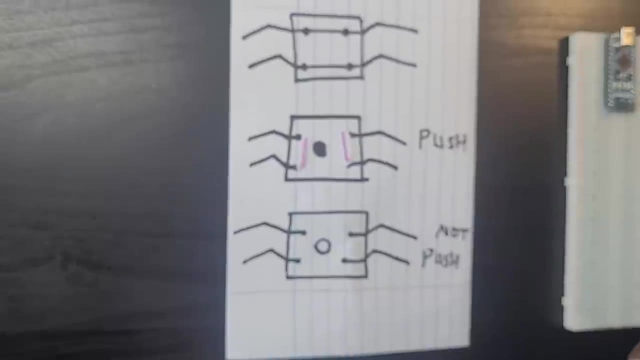 the same side we're gonna be looking- wait, let me just focus here. the same side, we're gonna be looking for the same side. so they're always what they're always connected to. what they're always connected. let me just focus again. they're always connected to what? in the condition that we push. 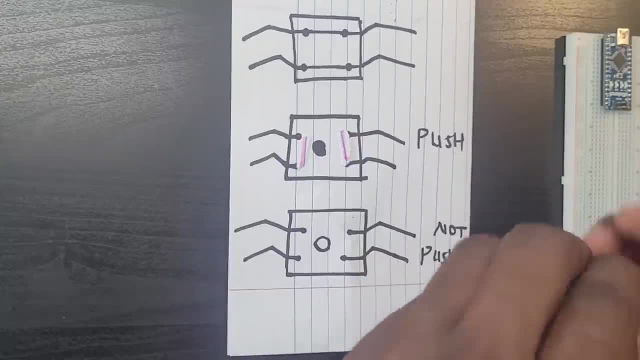 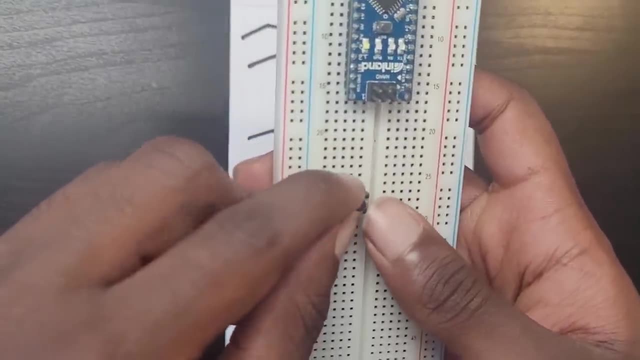 this is where the switching occurs again. so i have to connect them in what i have, to put them in a way where the same sides are what they're in opposite, what they're opposite rows, they're in what are different rows. okay, let me just do that. let me. 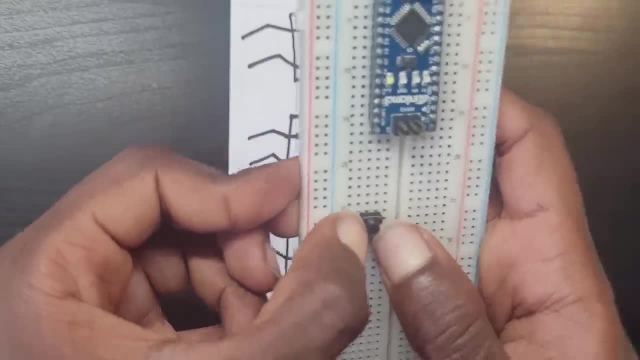 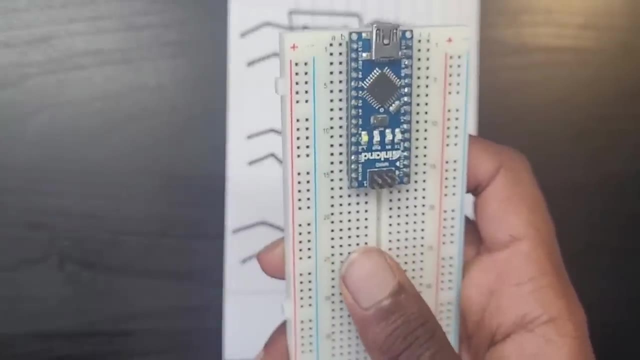 just put this in the middle around here: connect that, push it again. you have to push, by the way, these buttons. they take a lot of effort and you have to push them. just make sure that you don't break them. okay, there we go. just do it gently. okay, now i can do is what connect my arduino. 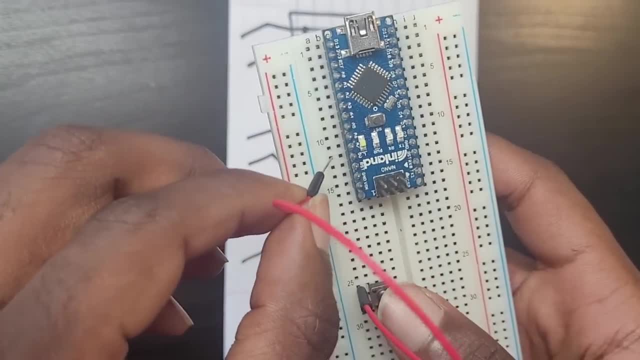 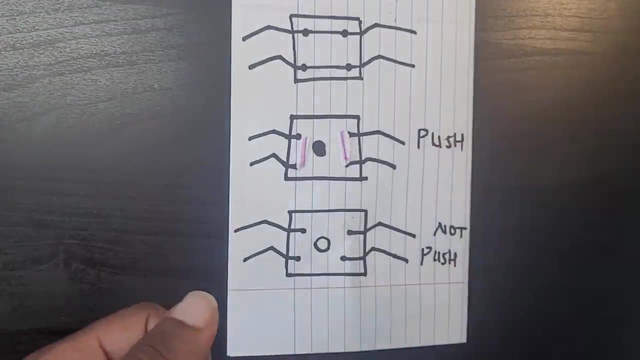 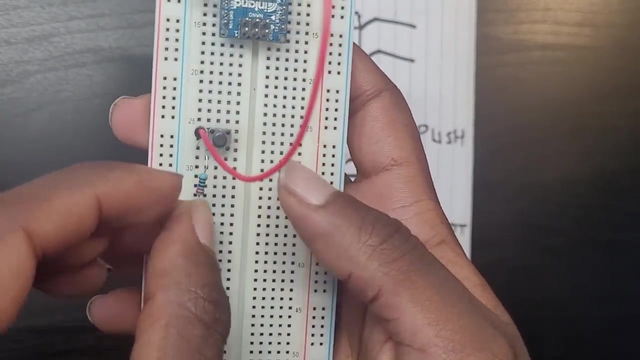 does the all. right, let me just go here, actually connect to the five volt right here, all right now. what do i need to do? my resistor, let me spring my handy resistor here, and i need to do is put it what across again. i'm going to put it right here across and what do i? 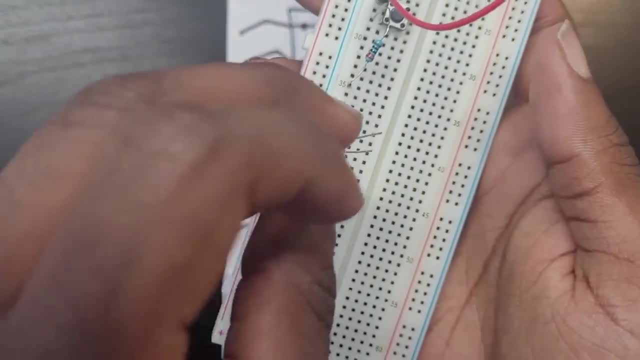 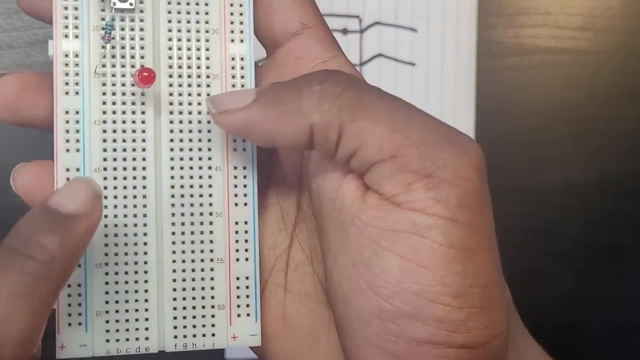 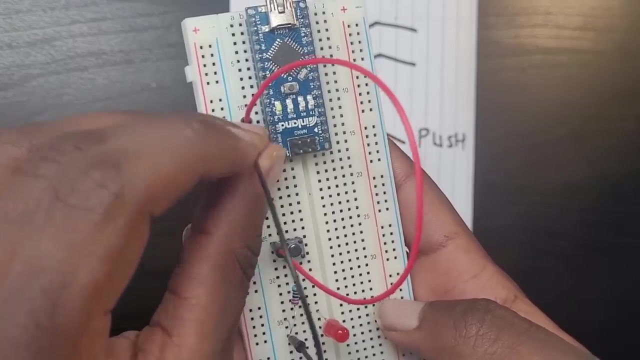 need to check that. you know, obviously the current is moving or not. leds: we're going to be using our handy leds and then we're going to be obviously using the gnd. we're going to be connecting to what? to the gnd right here. so i need to connect this to what? to the g and d. okay, 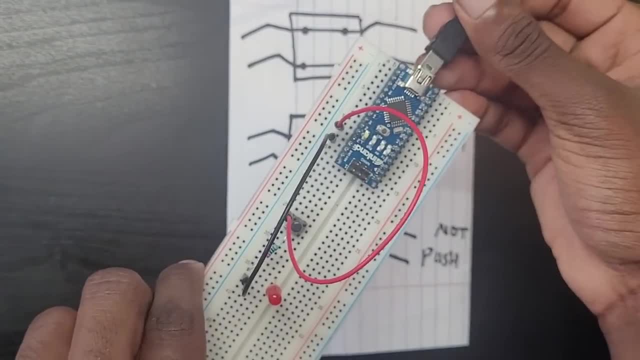 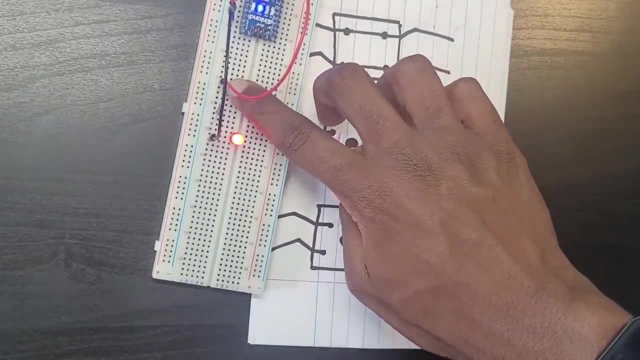 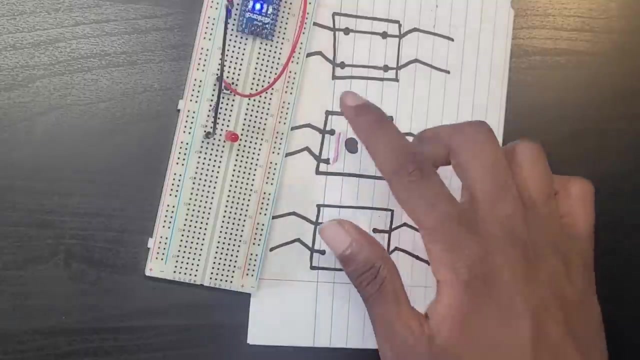 so now switching should occur. there we go as soon as we push. again, what happens? as soon as we push, it starts to turn on, but as soon as we let go, it turns off. this is where again, where what happens the switching occurs. so the same goes for the gnd. like you're going to play this right here. you're going to play this here. 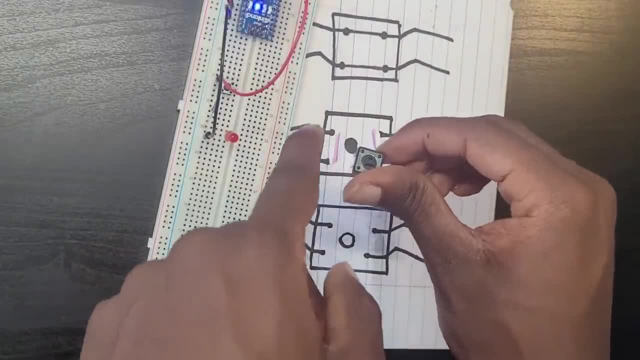 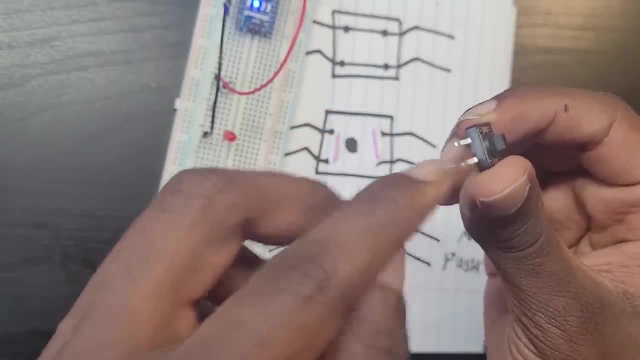 this one too, it's exactly the same thing. all right, the switches are exactly the same- push button switches, but the only difference is what: their size and, again, their leg placement. okay, so if you always look for the sides, again, don't look for the ones that are far, again far and uh, closer, don't. 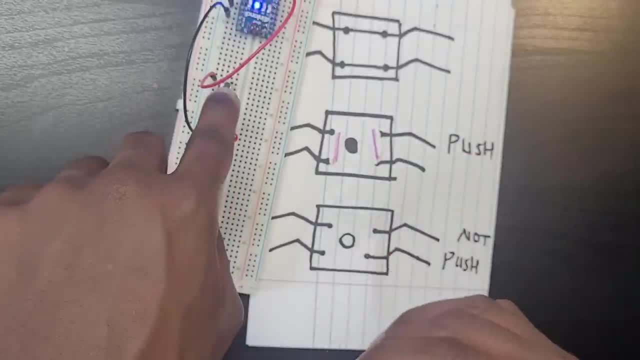 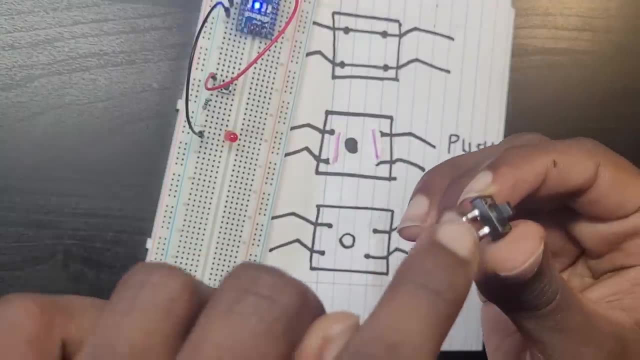 use that reference, because this one does not work here, because this one is a square, okay, so there's nothing called far or uh, close, because they're equally distanced, all right. so you always have to look for what for the pins that are on the same side, when they're on the same side. this is. 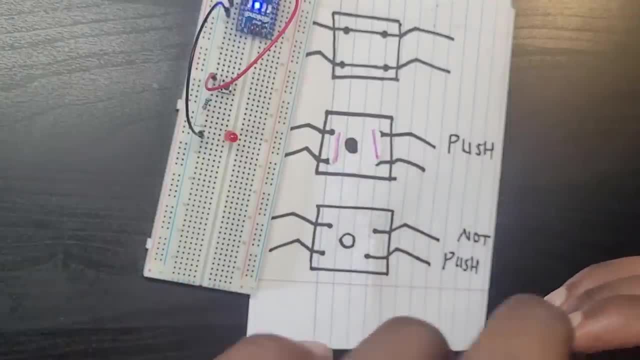 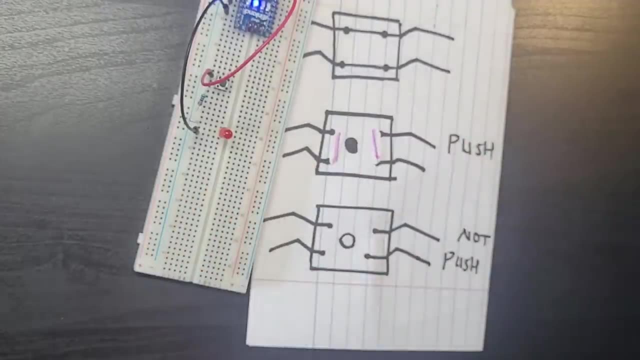 where the switching occurs and when they're what? where? when they're on the parallel side, what this is what they're always, what they're always connected. either even you push it up or don't push. so just keep that in mind before, uh, moving on. all right, that's all when it comes to switches. 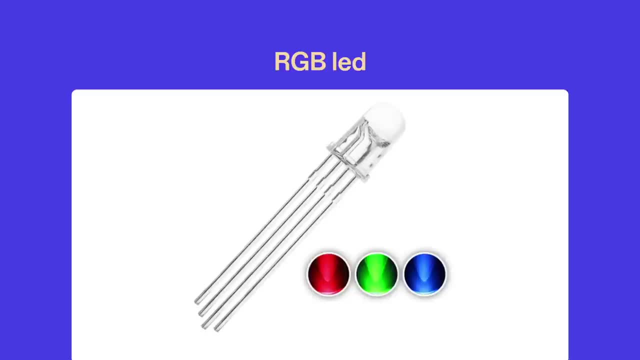 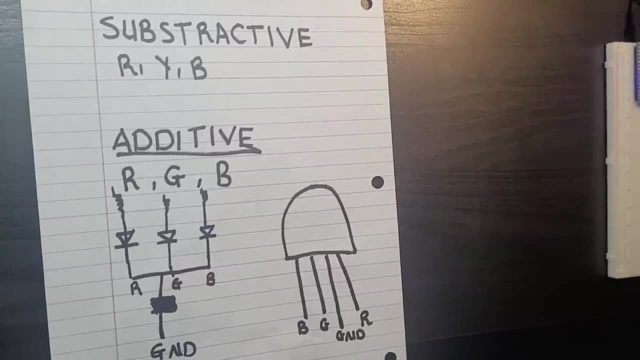 so, um, see you in the next section. okay, so in this section we're going to discuss about leds. we work with leds. we've put lots of leds in our project, but we're going to be discussing about a special type of led. so we've worked with the, the red led, the. 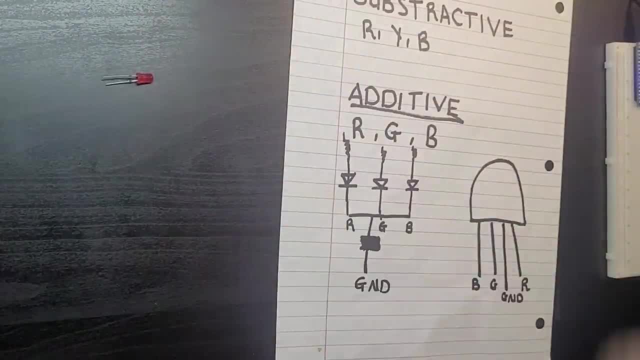 most, but we also worked with what? with the green led and also the yellow led. we're working on the traffic light project, as you remember. right here, the important thing i want you guys to know is: all right, let's see, we have a green led right here. i have a green led right here. all right, that's good. 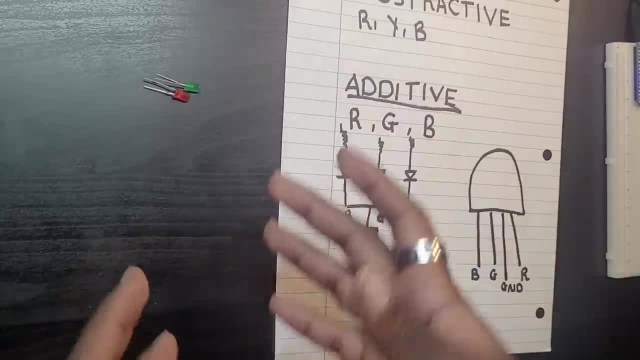 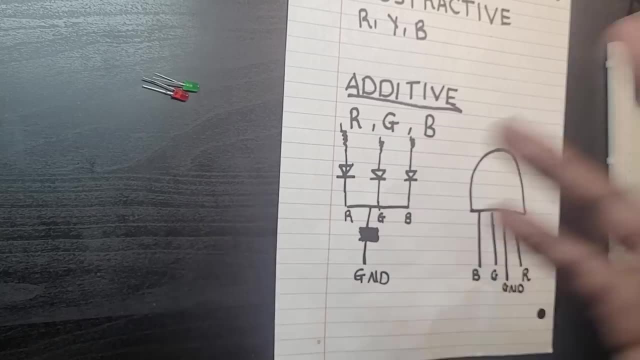 what if i want a pink led? what if i want a purple led? i have to specifically buy what an led that is purple. i have to specifically buy an led that is pink if i want the pink led, that creates. what a problem. okay, so how do i get any color that i want in an led? this is where rgb leds come to place. 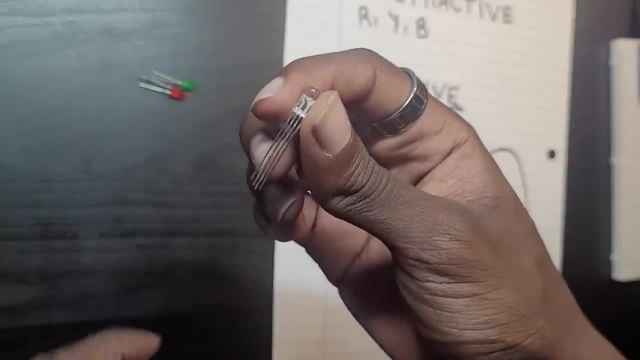 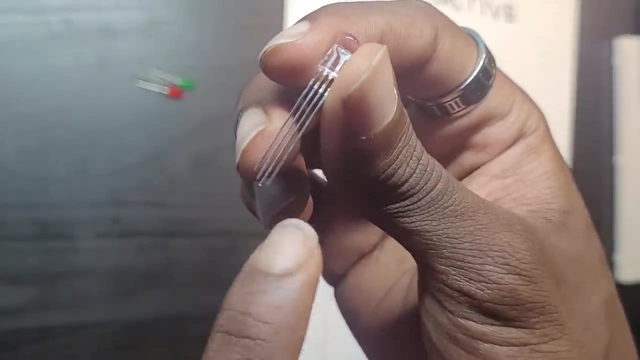 okay, they are called rgb leds, and if you want to find them in your kit, one thing you have to look for is that they have four legs. okay, they have four legs. let me just focus here. they have four legs. not only that, too, but even the third leg right here. the third leg is a bit longer, okay. 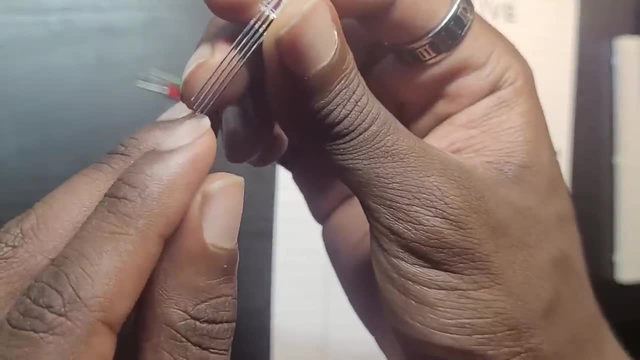 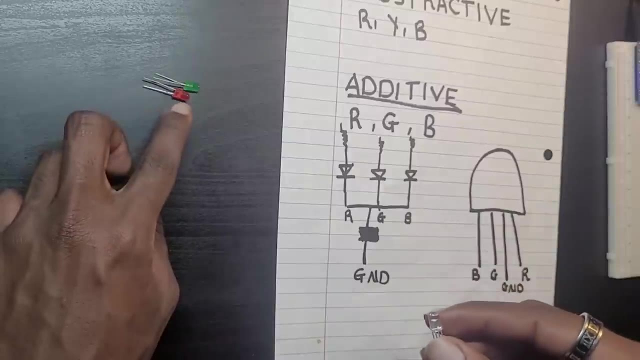 i'm going to get to why. it's longer, but there's a third leg right here that is longer, so we have to look for something that has four legs and looks like an led. it has to be clear, okay. it doesn't have any color, just like how these leds used to. it's going to be clear, okay. so what are these rgb? 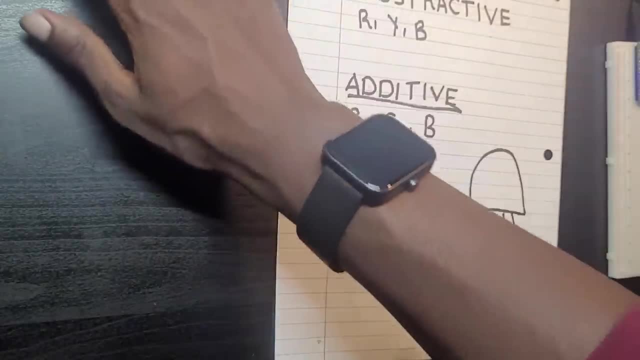 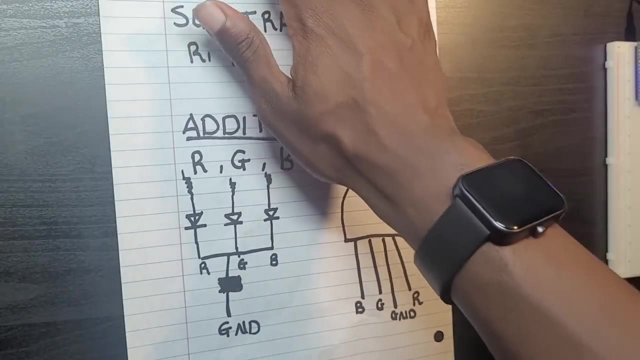 leds. before getting into that, i really want you to understand the science between color, all right, so we have to understand. we have to understand the basics of colors so that we're going to understand. how does this rgb led work? okay, how does this rgb led work? okay, so to do that. 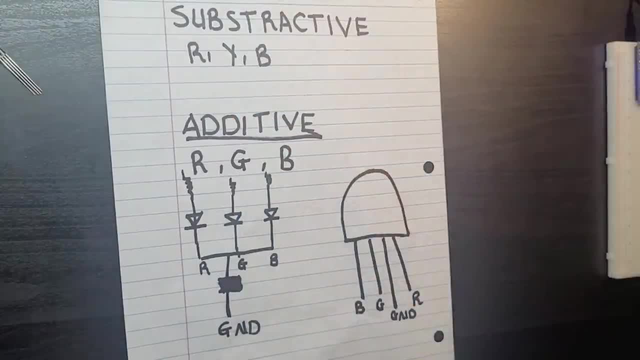 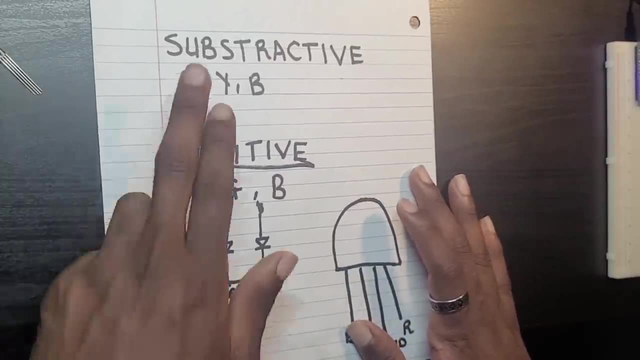 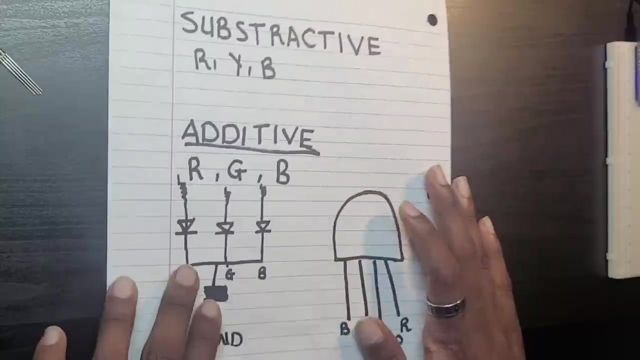 let's just discuss about something very, very, uh, very, very basic. okay, so i think most of us by now have learned that, um, the three primary colors are what? red, yellow and blue. i'm correct, we've learned that the three primary colors are red, yellow and blue. all right, right here, though. 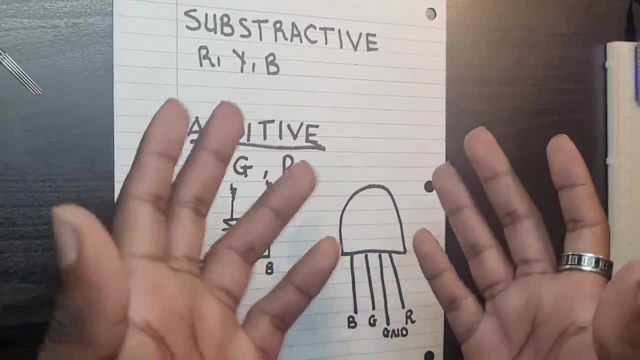 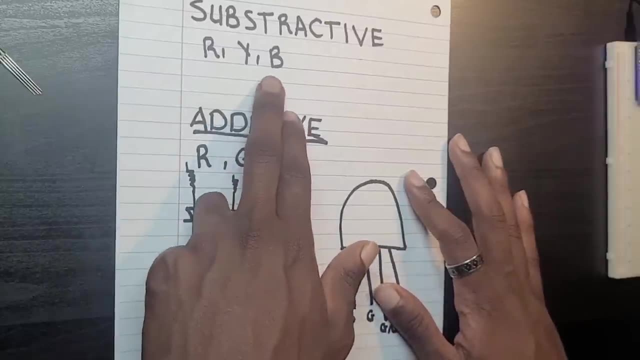 we're not going to be using red, yellow and blue. we're going to be using a blue and blue color and we're going to be using a purple and a red and a blue. so basically, what does this mean? these three primary colors, they can combine to create. 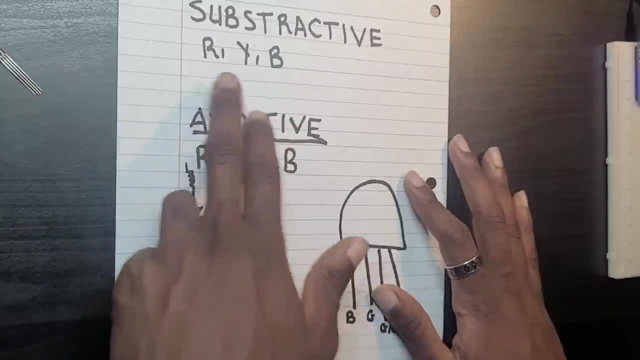 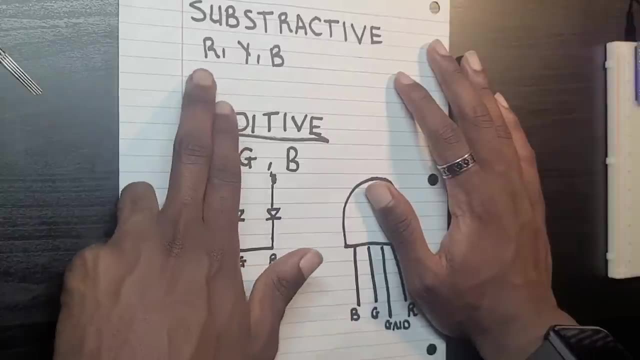 any color that you want, any color that you think of. yellow and blue together gives us green, red and yellow together gives us- uh, it gives us orange, red and blue gives us what red and blue gives us, um, purple, and even, you know, even putting less red and putting more blue is going to give us more. 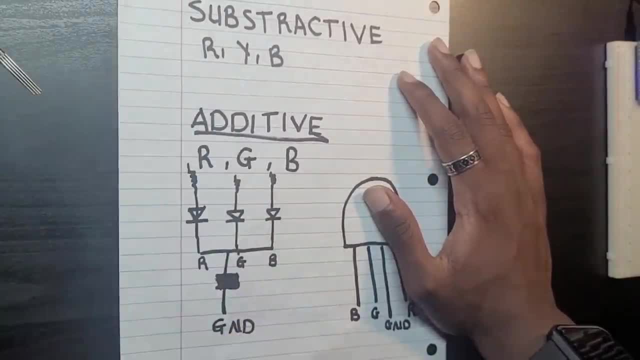 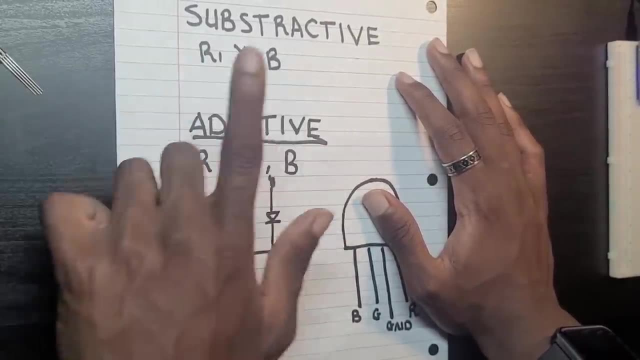 purple, little bluish looking type of purple, you know. and it keeps going on. so the list keeps going on. so let's just look at what we want, from black to white to purple, to any color that you're thinking of. can be made from what? from the combination of what? these three primary colors? 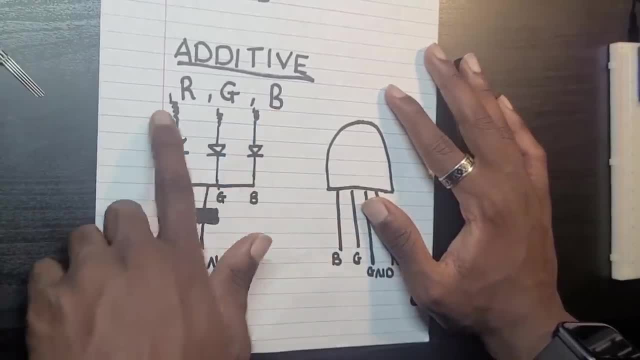 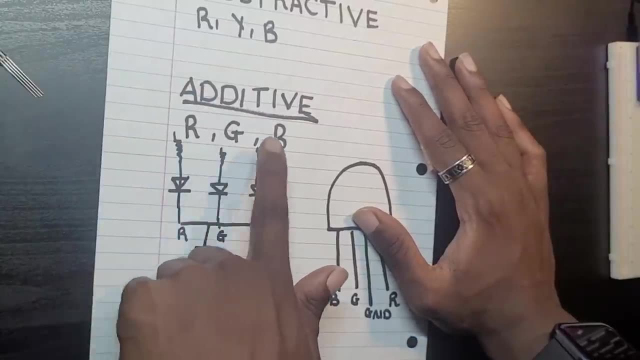 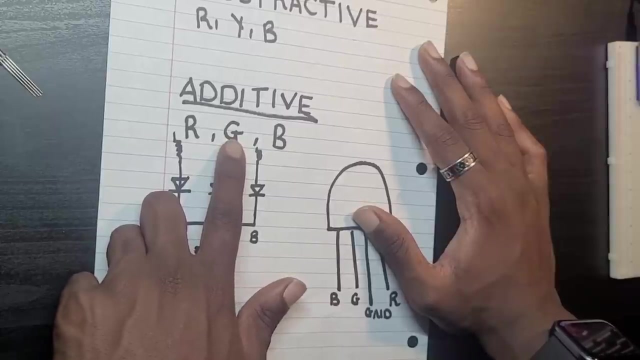 okay, but we can also do it using another color. instead of yellow, instead of yellow, we can also do the same thing by using green, by using red, green and blue. we can literally create the same thing when we connect a red and green. what do you think happens when we connect red and green? 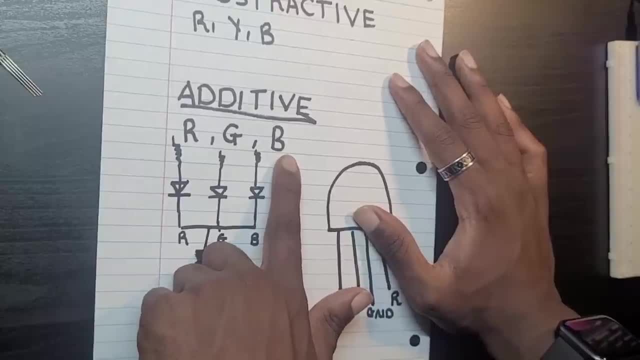 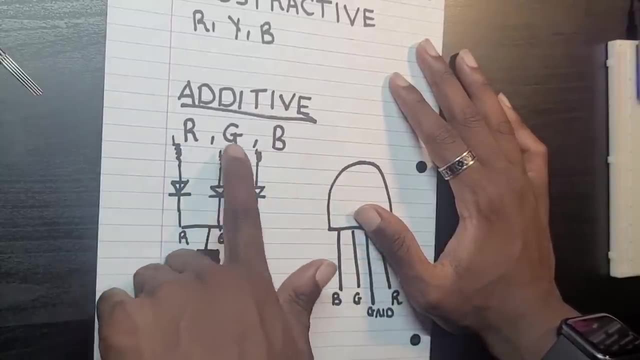 to be honest, i really do not know. when it comes to red and blue, obviously, what happens is it's- uh, it's again purple. when it comes to green and blue, uh, it becomes cyan. i don't know what happens when you connect, uh, red and green. i don't remember. 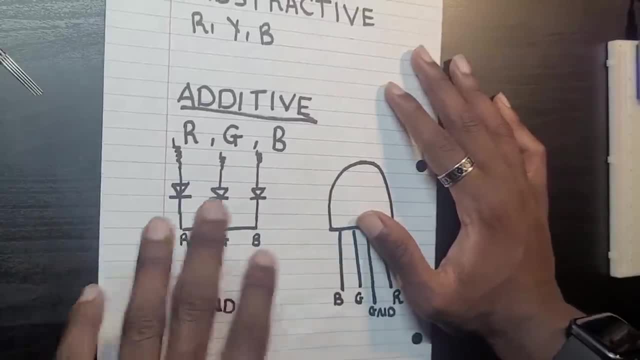 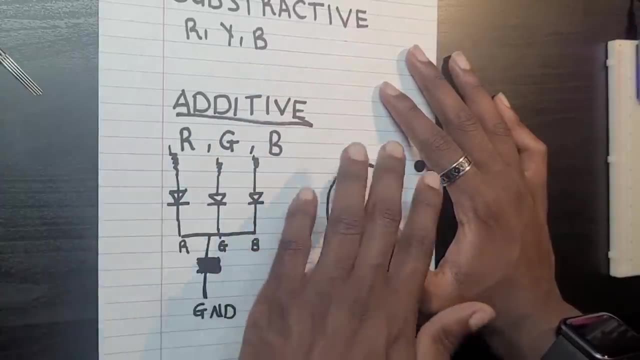 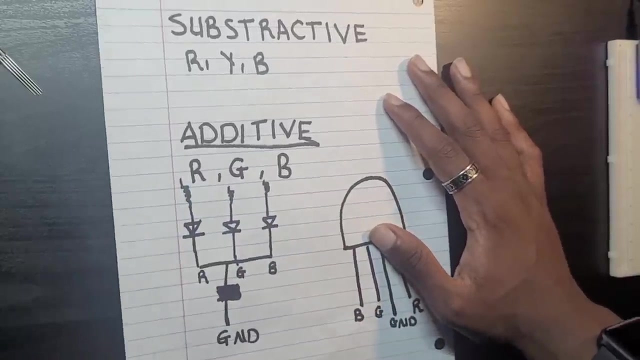 i really don't remember, but anyways, the main thing is it exactly does the exact same thing that we just mentioned here. it can create any type of color, can create any type of color that you're thinking of again with red, green and blue. they can be what primary colors? so you might be. 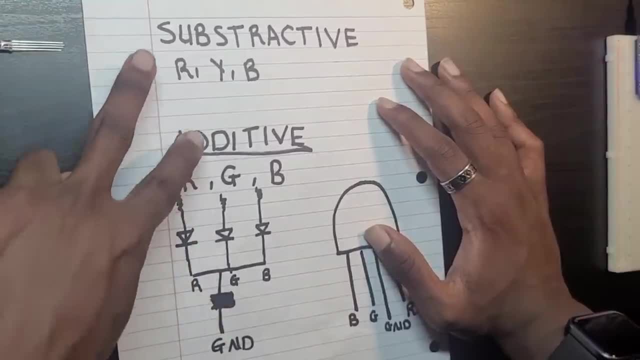 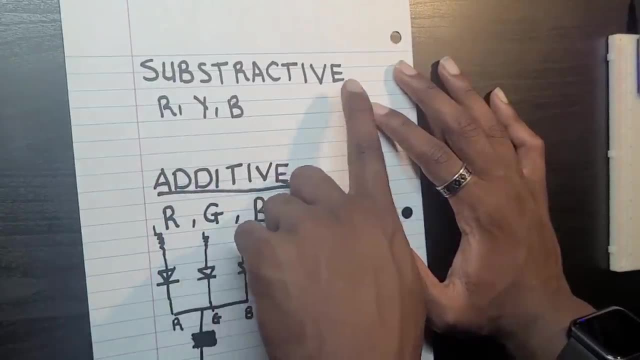 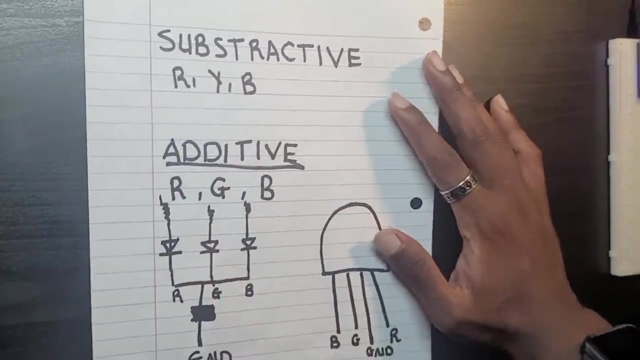 wondering: okay, which one are we going to use when we're working with this led and even with computers? so let me just go over right here. they are known this red, yellow, blue- are known as subtractive, subtractive colors. why is that so? i want you go. i'm just going to go over to my screen. 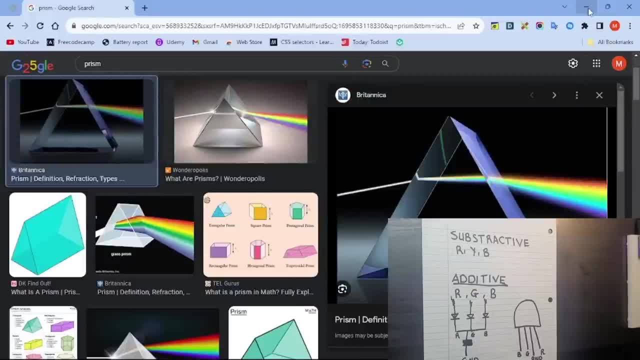 and try to explain it in a simple way. okay, so i think most of us know what a prism is. okay, so what does a prism do? basically what? it basically converts the sunlight right here that comes from the left side, to what? to a rainbow. okay, so what does it do it? 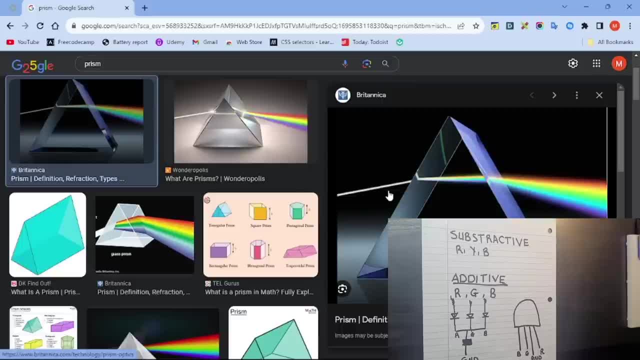 separates light. it separates it into different wavelengths or different colors, so that you can see each individual, each individual, what each individual, uh, color that makes, what that makes the sunlight, right here, the sun. okay, so one thing i want you to understand here is that it's called: 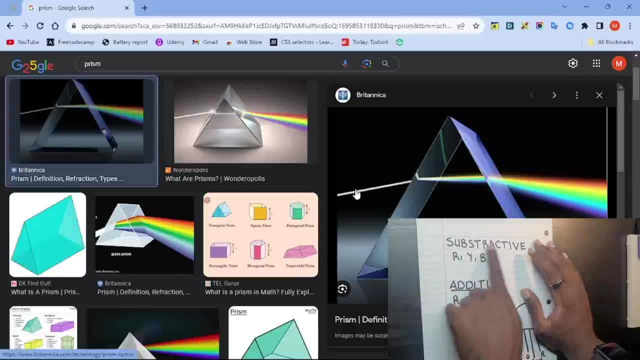 subtractive for a reason. what happens is what it is created by what by subtracting, so what basically happens, what is created by what by subtracting wavelengths of light, so basically what it's basically created from what by splitting light. okay, by splitting light, that's what happens when we're using a prism. basically our day-to-day life, when it comes to our 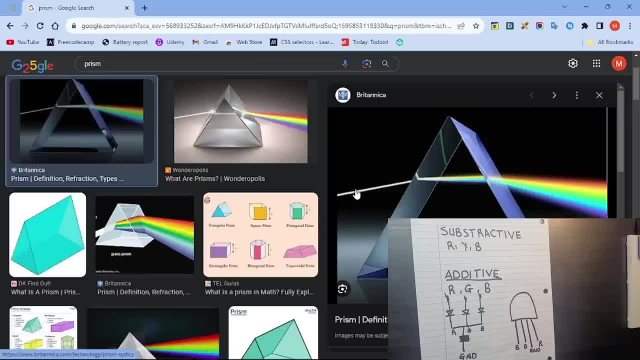 day-to-day life. obviously, we gain light from what? from the sun, so almost everything that we're going to be using is what is going to be red, yellow and blue, made from these three. all right, because again, what are you going to be separated? and then what happens? and then, when it's separated, again we can. 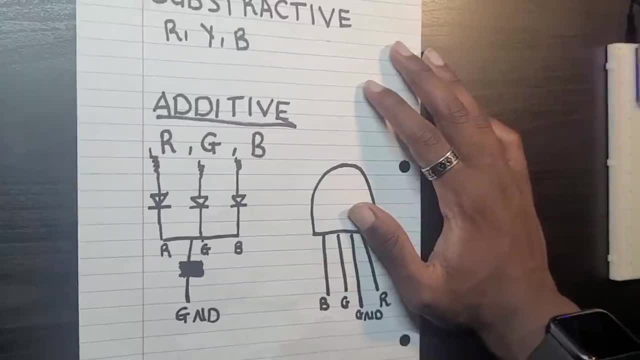 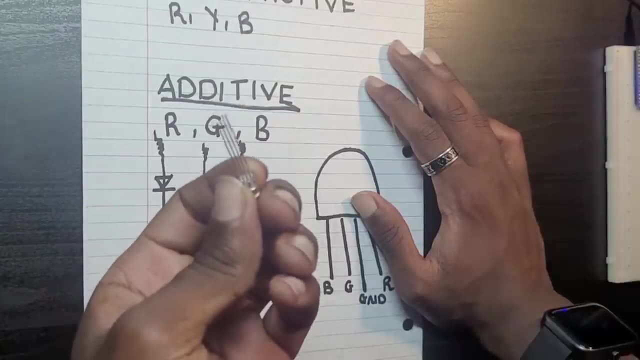 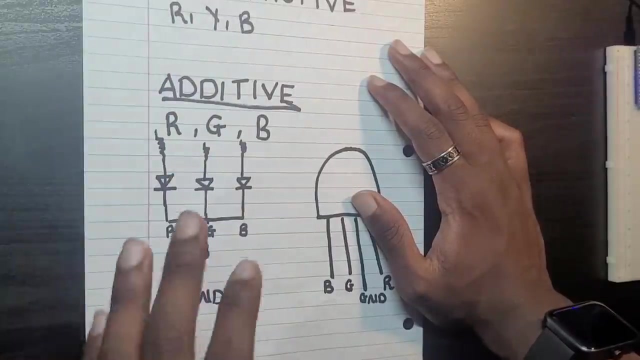 see colors, all right, different types of colors, okay then. when it comes to the computer world, though, there is a problem. we use something called rgb. even the name of this led right here it's known as rgb led. it's known as what: r-g-b-l-e-d. let me get to why we use rgb instead of ryb, and 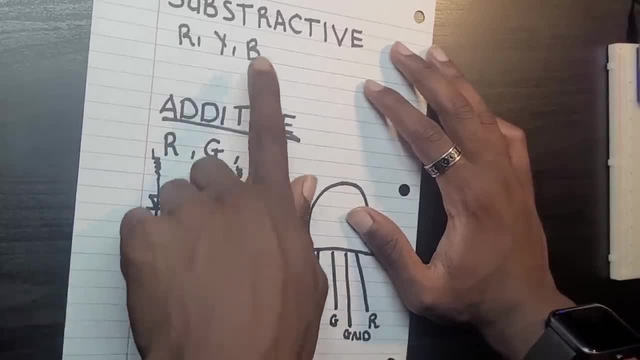 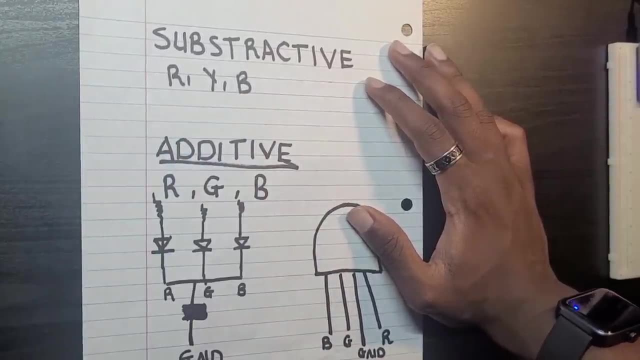 what in our computers. so the problem here is light. okay, when it comes towards subtractive- uh sorry, subtractive- colors, they have to first gain light and they separate it. so they gain light from the sun. what do they do? they separate it. okay, they separate into different wavelengths, or basically different colors of light. okay, when 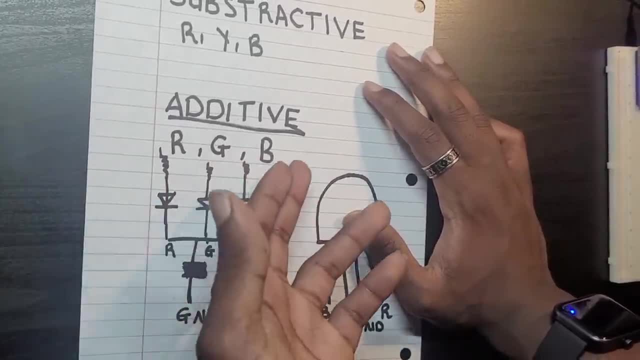 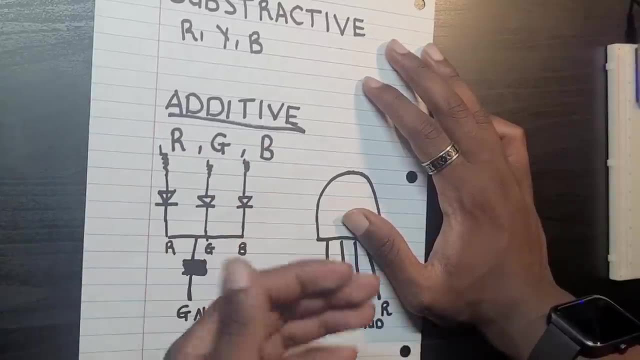 it comes to additive, though. why do we use additive in computers? is we don't use the sunlight. that's the problem. our computers do not use sunlight. where do they harvest energy? they harvest energy from what? from electricity, basically, when we charge our phone, when we charge our computer. 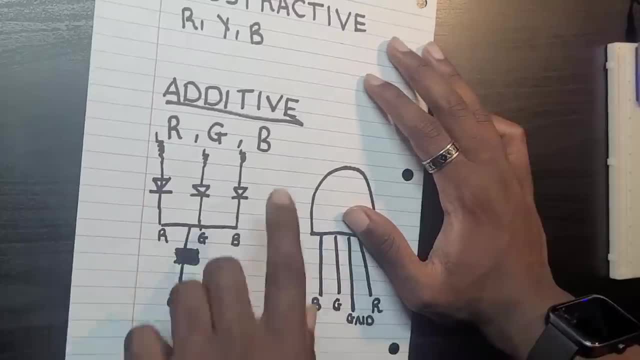 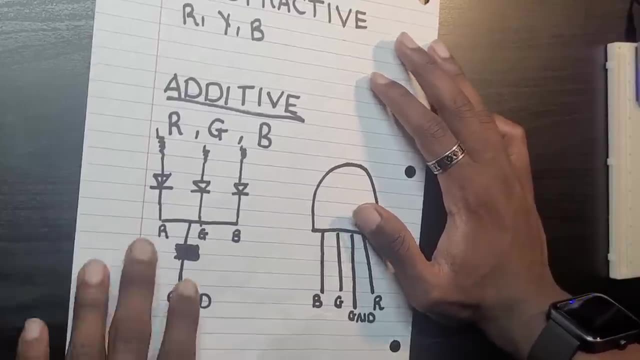 when we charge, obviously, our devices. so right here we're changing electrical energy. to what? electrical energy into what? into light energy. this is very, very important. so we're not what, we're not big, we're not going to be using a light and then separating, and we're not going to be 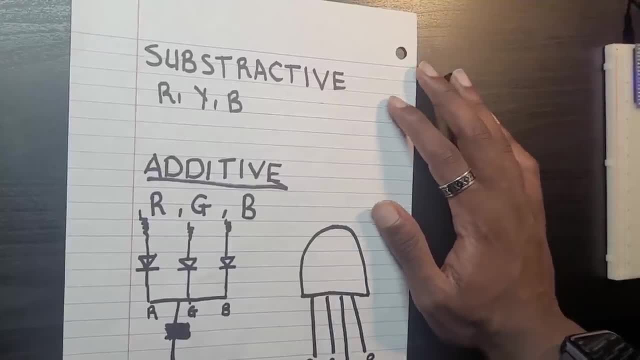 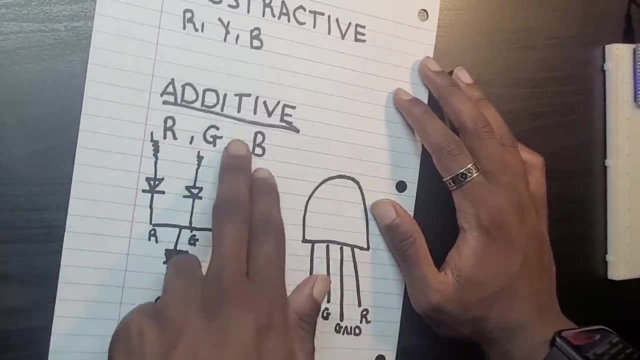 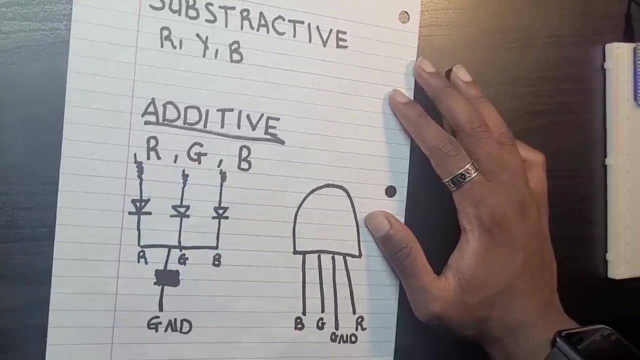 gaining light from somewhere and then separating it. obviously, when it comes to our devices, they don't. what we don't use, uh, we don't use sunlight, obviously, to charge our devices. that's why we don't use subtractive or subtractive color, obviously. so right here we're going to be using additive colors. additive colors is literally the. 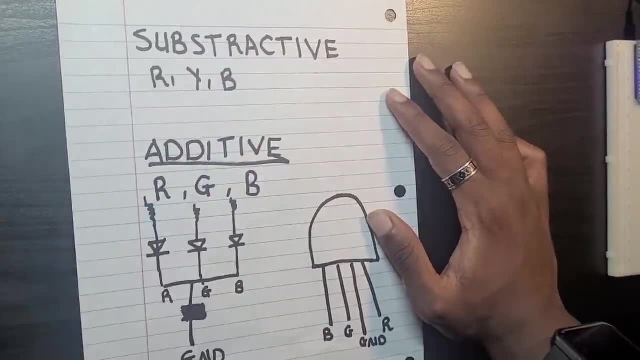 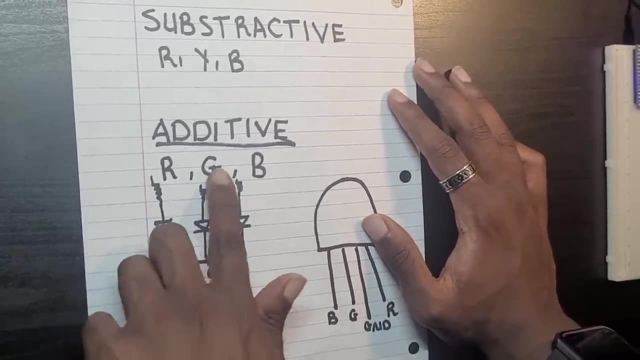 opposite of what i said, subtractive. when i say subtractive, what do you do? we split. so, basically, when it comes to rgb, what do we do? we combine. you see that we combine these wavelengths of light to create any light we want. so we're gonna what we're gonna: combine them. that's the very very 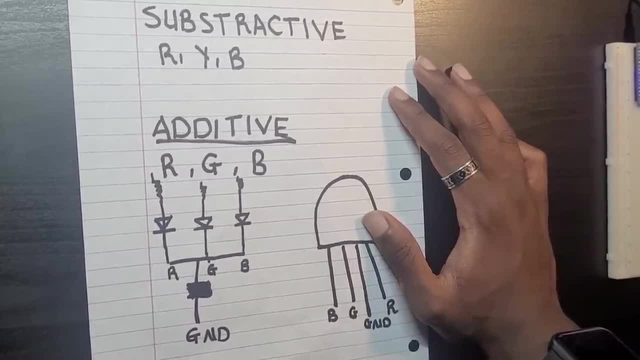 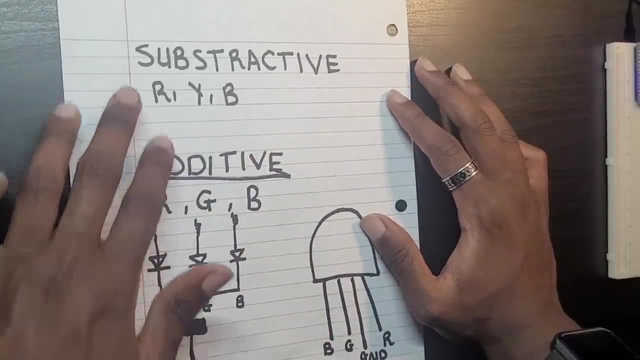 important thing: we're gonna combine them. and when you combine them, what do? what happens? we're gonna be creating every color that we want again, so we can find again ryb and rgb. the fundamental difference between them is: what is again this separating light and this one what adding light? 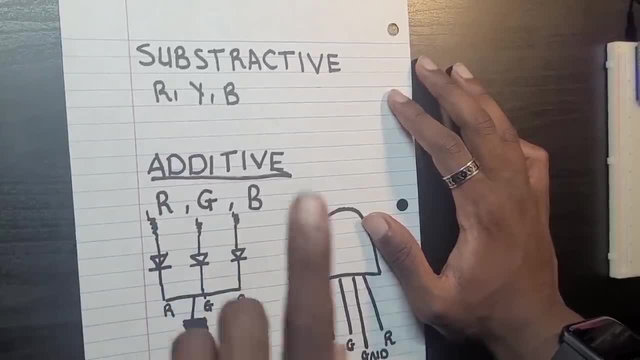 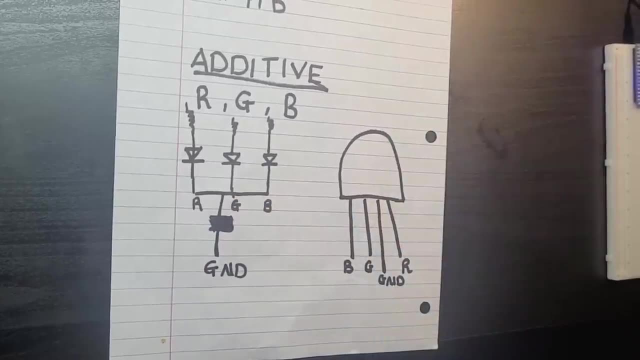 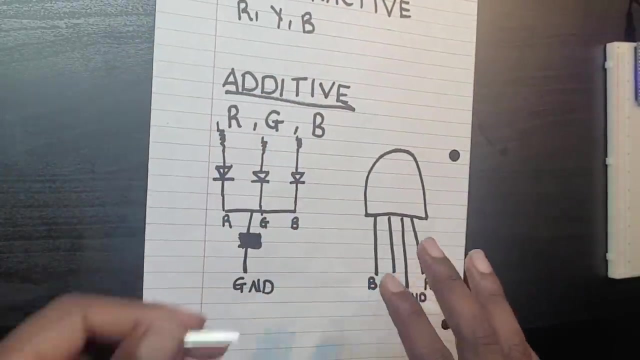 okay, this, what blending light? okay, and it's very, very again important, what in computers we're going to be using rgb? okay, all right. so with that in mind, we have to first, uh, try to actually work with the led first. so let's try to understand this led right now, and we're going to go and understand. 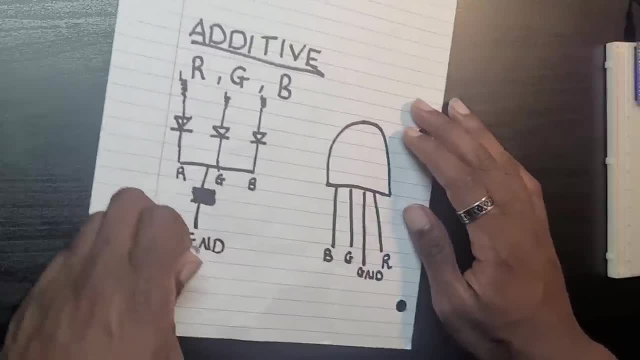 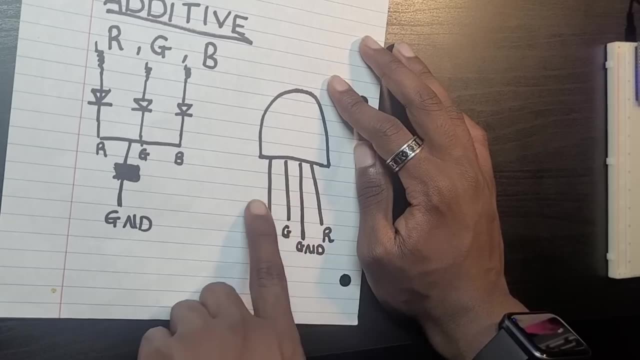 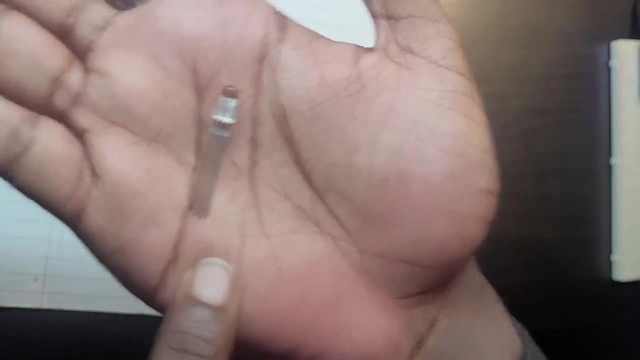 how the inner parts work. okay, so when you look at the led, it has four legs. as i said again, one leg is always what. the third leg is always longer than the three legs. so the fourth leg right here. let me just bring it right here, i think. let me just focus it all right, let it focus the fourth. 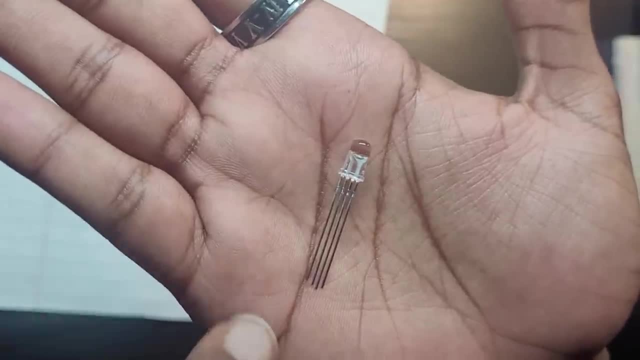 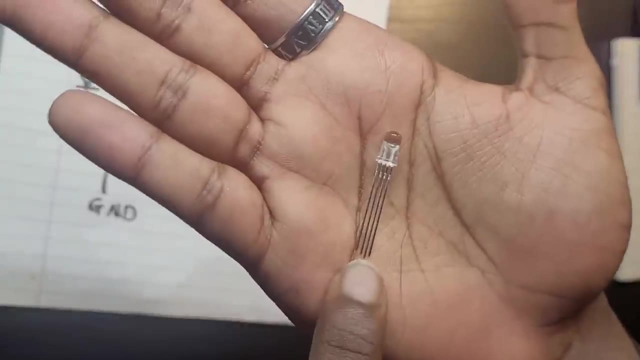 leg, as we can see right here. let me start from the first one. the first, the what the most left leg. basically, the first one is what? it's going to be blue, okay. and the second one is going to be blue, it's going to be green. the third one is going to be connected to the gnd pin, and the fourth one 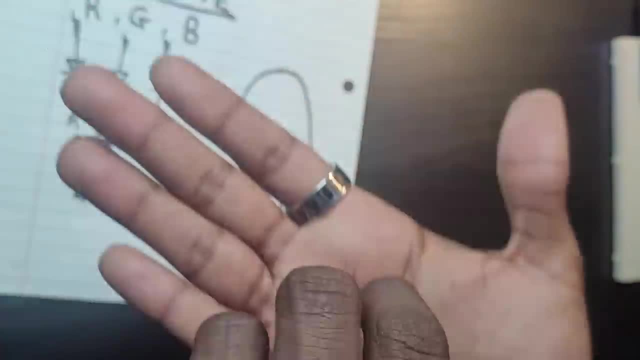 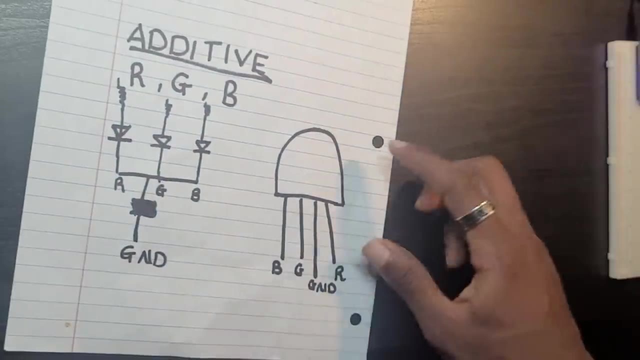 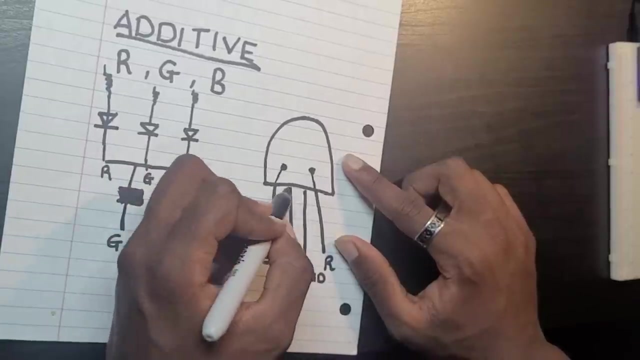 is going to be connected to what it's basically the red light. okay, that's what i want you to think of them, okay. so one thing you also need to keep in mind is: okay, this is going to be, let's say, a light compartment. right here, there's a blue light compartment and there's a green light compartment. 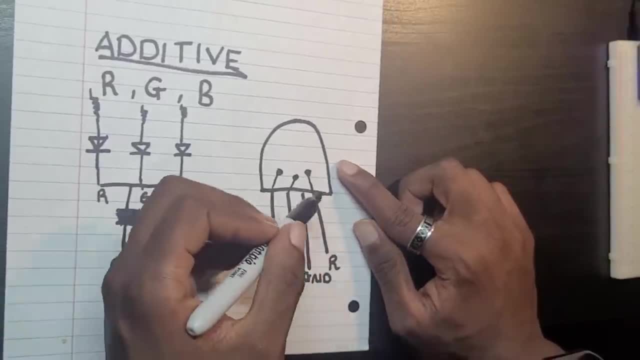 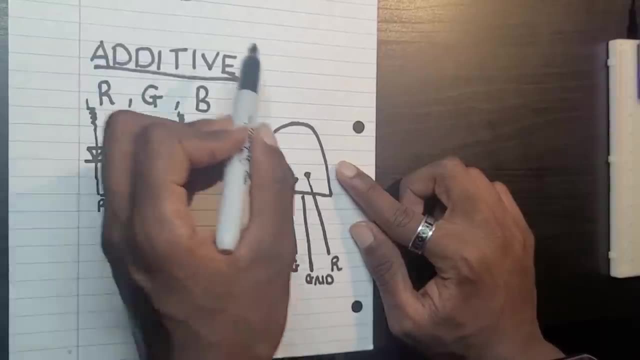 right here. okay. so basically, what happens, as i said again, when the red turns on, for example, the red is on and the blue is on, what happens? we get a purple. okay, because it's again an additive we have to add up together. we add up lights. okay, when you add red and blue. 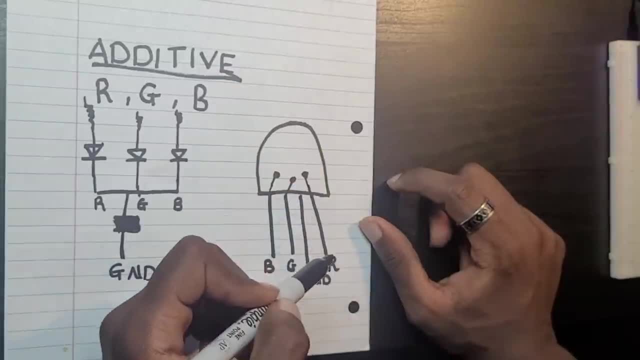 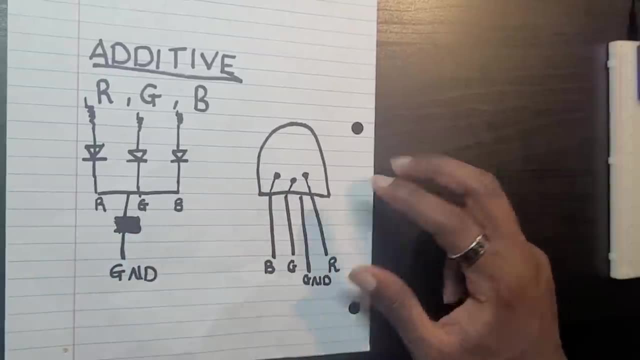 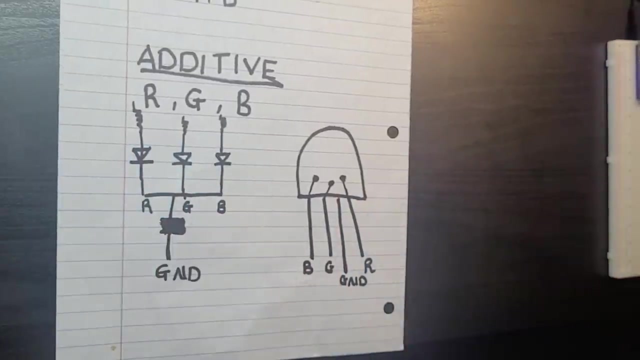 what happens? we get purple right here. so let's say it's just basically what turning on red led and the blue led, what blue led? when you turn them on, it's purple. so i want you to think of them as combining three leds, combining red, green, blue leds into one led. okay, just think of them as. 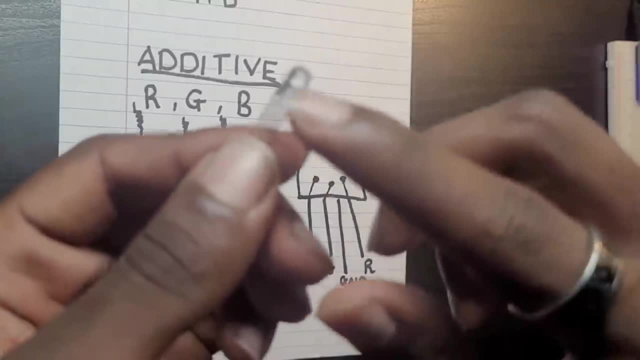 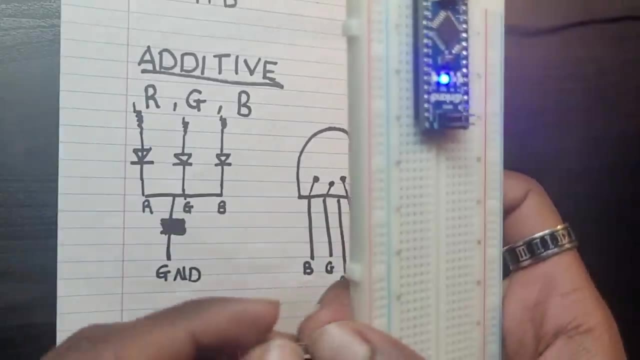 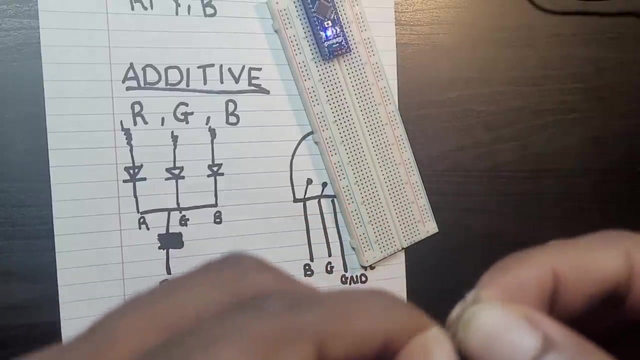 combining three leds into one led and fitting them in this space. okay, that's what i want you to think of, that, okay. so what's going to be interesting is actually- let me just put this again across- it's going to be more interesting if we learn as we go. it's better that way. 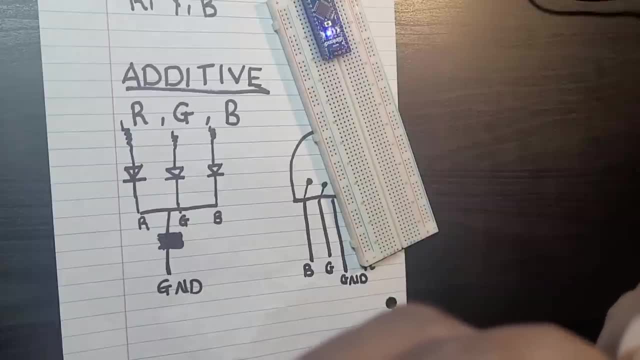 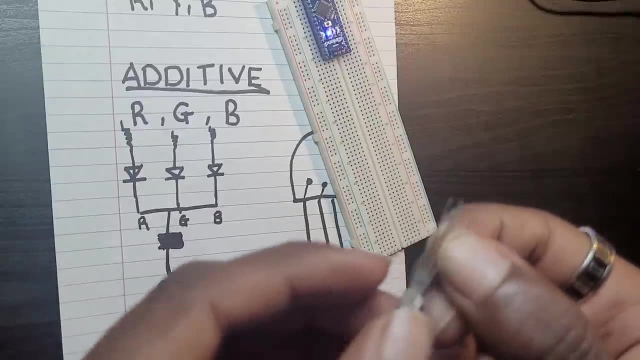 so you guys can actually retain the information. okay, let me just open this. i need to pry it a bit open because it's not going to fit across. i don't do that. all right, that's better, i have to just keep track of it. the third leg: let me just again focus on this one. 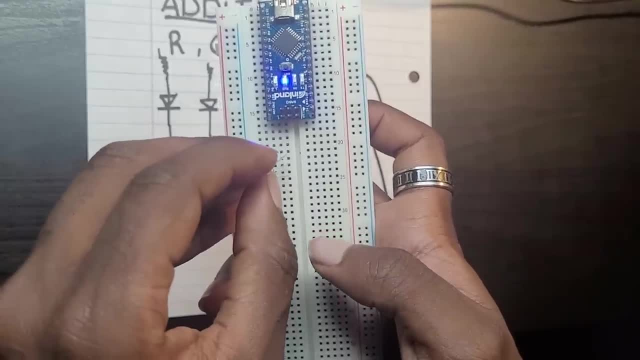 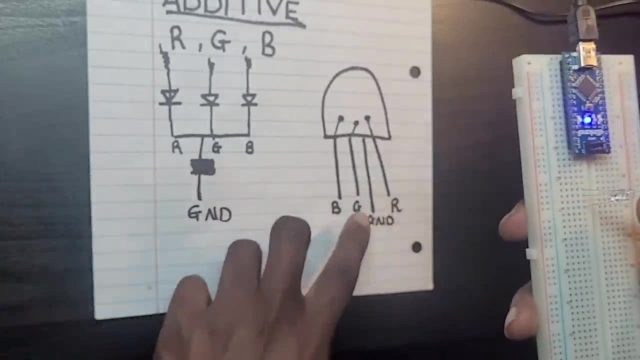 i'm just going to keep it like this. the third leg is going to be here, the gnd. you need to make sure which leg you're putting. okay, this is the first one is what, the blue, the, the most left one. the second one is green, the third one is gnd and the fourth one is what. the fourth one is r. 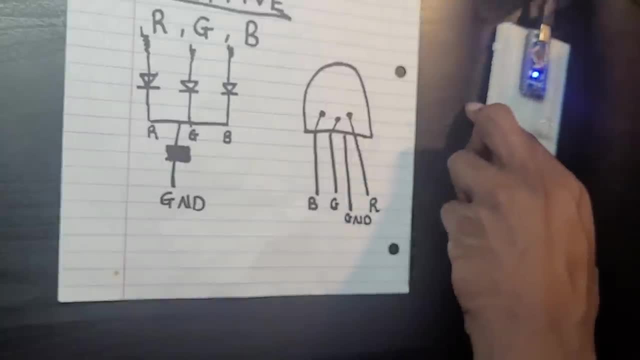 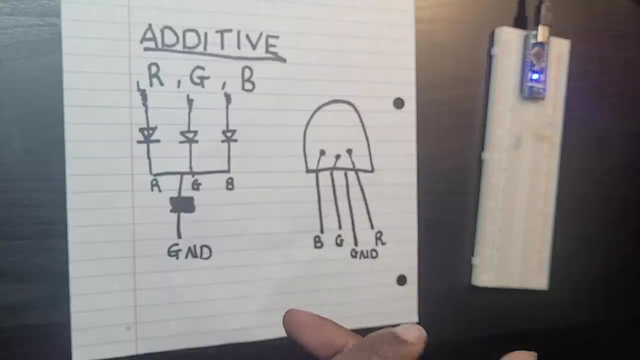 all right, that's how i set it up right now. so you might be wondering: okay, what is? is all this rgb? how am i supposed to, you know, find yellow? because right now i've only talked about purple, maybe creating a cyan right here, but i've not talked about, you know, finding any color. 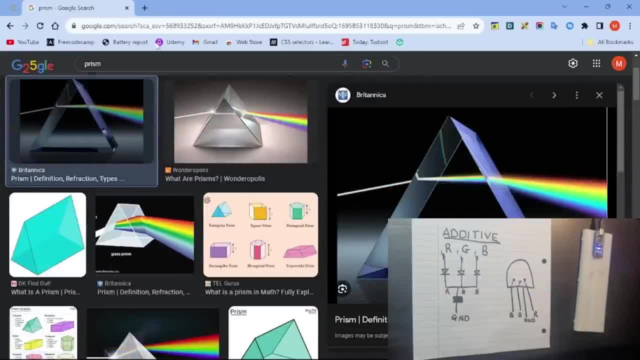 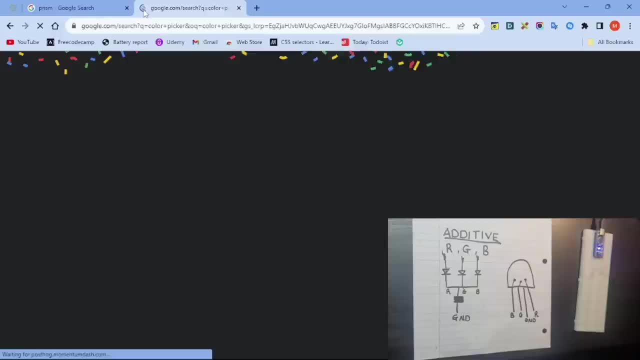 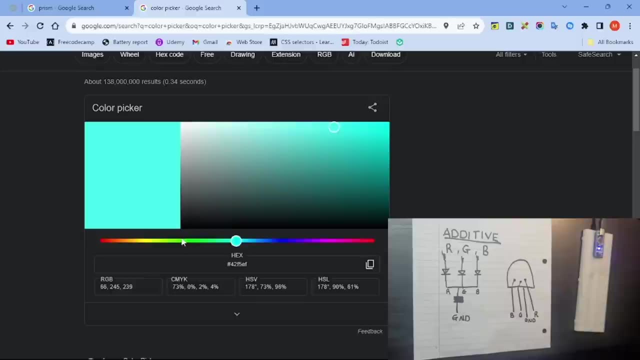 so let me go over to my screen right now. let me just do that, and what i want you to google is, say color code or color pick, say color picker, and even google has this. so all you need to do is basically choose any color you want. in this case, let me just choose green, for example. let me just say the, the 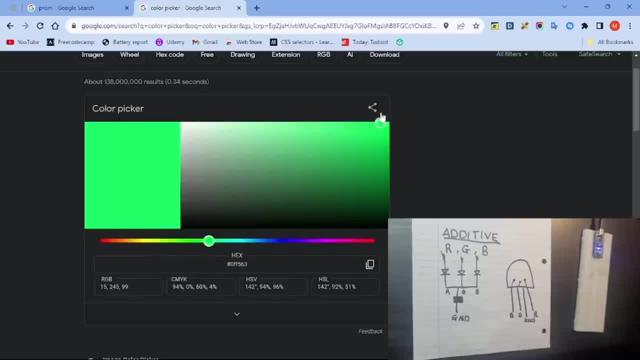 most green thing. let me just go to the most green one. just choose that. this is not the most green, this looks the most green. almost we cannot see the difference right here. okay, okay, this is the most green one because it only has green. right here, the green one is the. 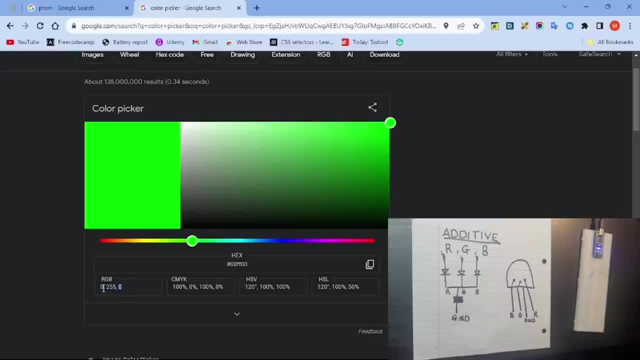 only one that's on. this one is all off, as you can see. this is off and this is the red one is off anyways. so you can just use any color picker right here and find the value here and you can understand the value. so you guys do not need to, you know, memorize anything. so you might be wondering. 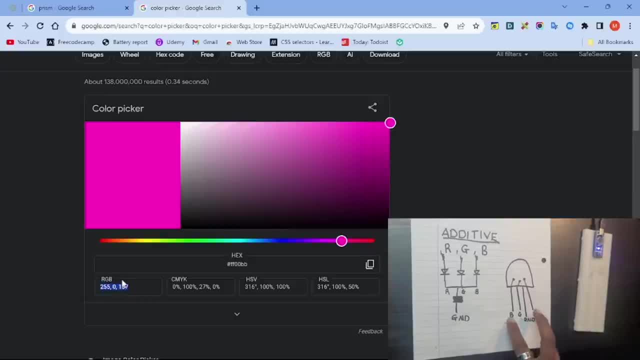 instead of: why are we supposed to, you know? call them rgb? why not just say you know? we can just say you know, if you want pink when i use the keyword pink. if you want, you know, purple, why not use the keyword purple, you know? doesn't that make more sense? you know, because it's going to be easier. 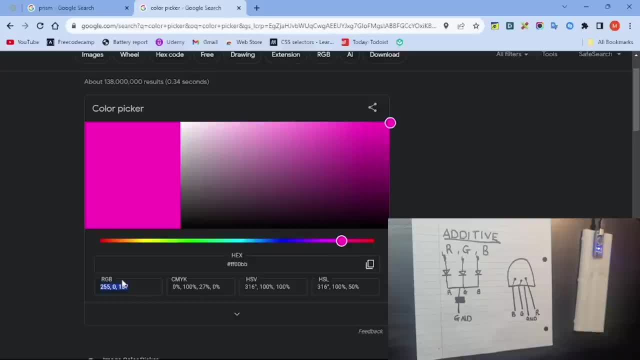 it's more easier, and you would have to create a whole new system for naming what? for naming lights, you know. doesn't that make more sense? i mean, it looks like it makes more sense, right, but the problem arises here is that the problem is that. the problem is that. the problem arises here is that 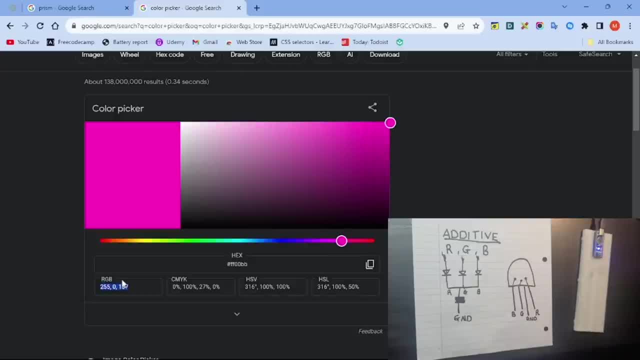 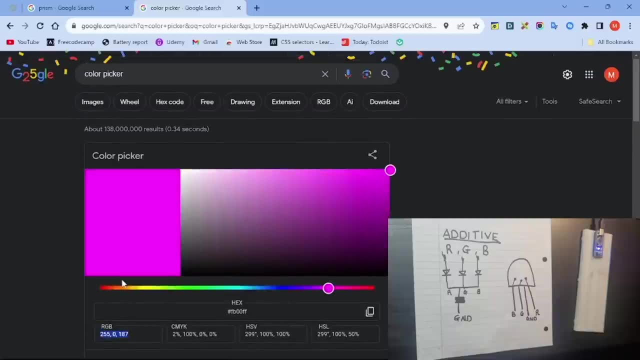 arises here. the problem arises is we have different combinations of colors- i'm talking millions to millions- combination of colors that even provides us in what, when it comes to the amount of colors we can even see. so, for example, let's say i want the shade of, uh, the shade of. 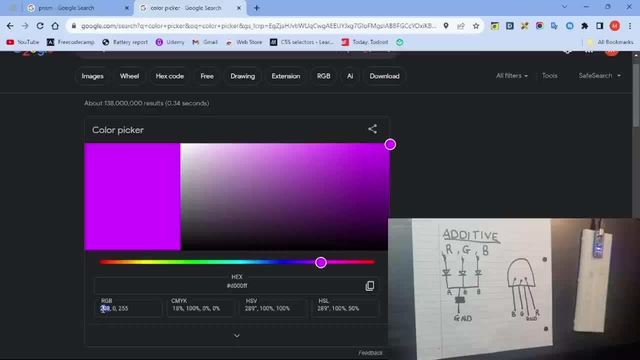 pink. i just, i just say i call it. let's say i call it pink 55. okay, i just called it pink 55. all right, i just give it a name: pink 55. then let's say, i move it a bit and i want it to be a bit darker. 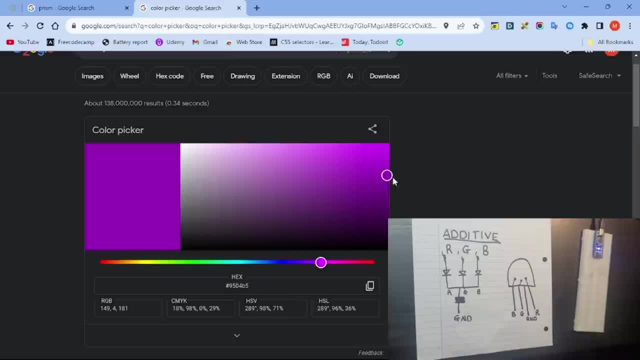 okay, i have to call this pink 56. let me just say: okay, let me just call this pink 56. all right, let me go right here. pink 57, uh, pink 58. you can see that when we keep naming it and naming it and naming it, it's going to be what it's: a lot. you can see that, right, you can see that we cannot. 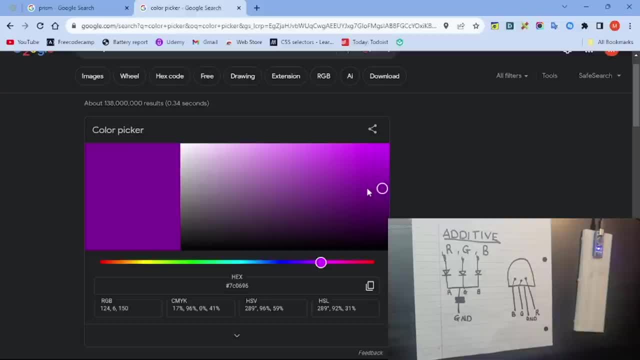 name millions of what? millions upon millions of color combinations, because why it's going to be infinite. the possibilities are what, the possibilities are a lot. so it's better to what to have a system and basically what direct ourselves. it's like, uh, i just want you to think of just just using a simple analogy. let me just get a paper right here. okay, let me just 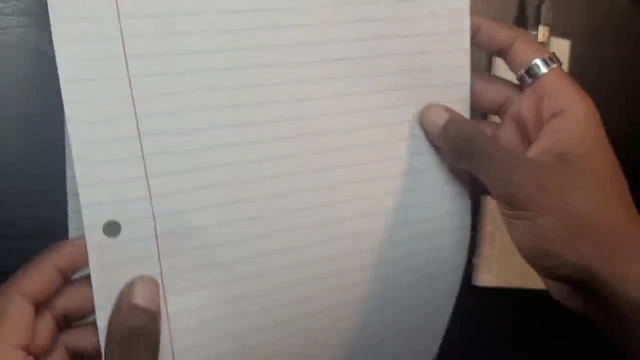 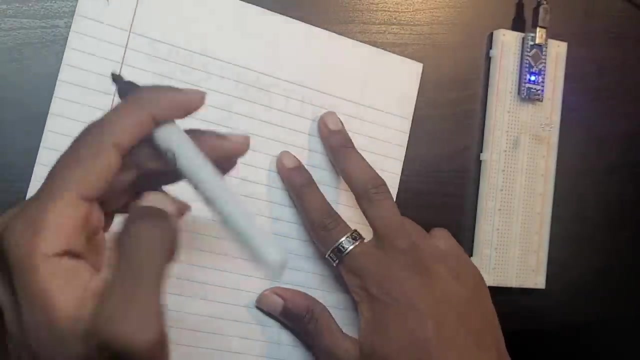 get a paper right here and let me just explain to you why rgb is important, why having a system of what using naming colors is important. let's just say, you know what you have to hold. one plus one is what two? okay, you have to remember this. all you do is remember this. you're not going to go. 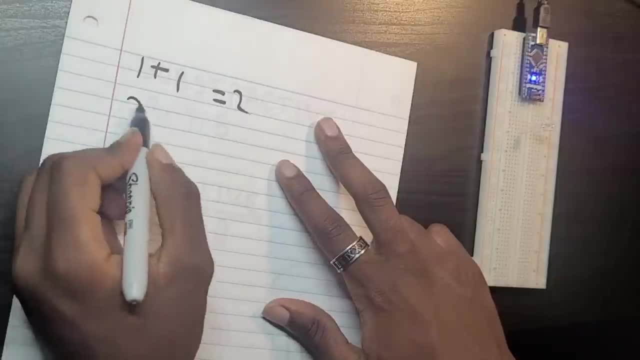 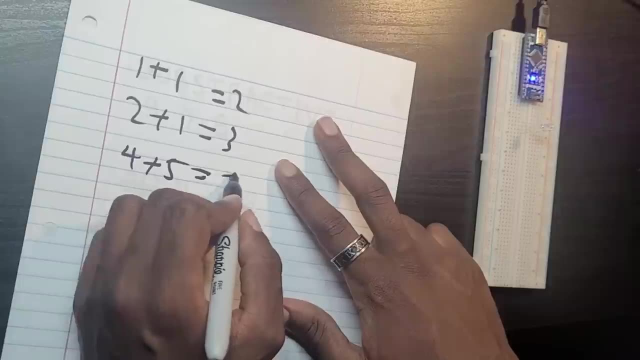 anything. one plus one is what it's true. we have to catch this in our mind: okay, two, two plus one is what three, uh. okay, four plus uh five is what it's. let's just say nine, um what? 10 plus 10 is what 20. 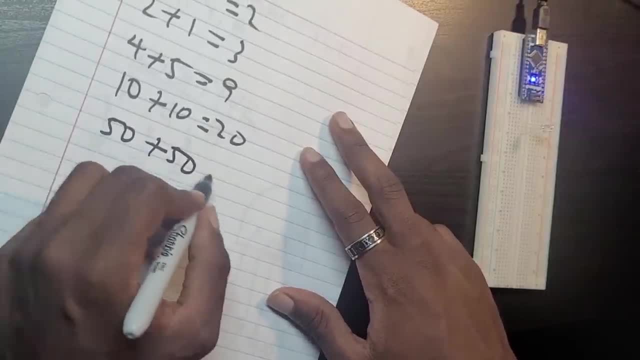 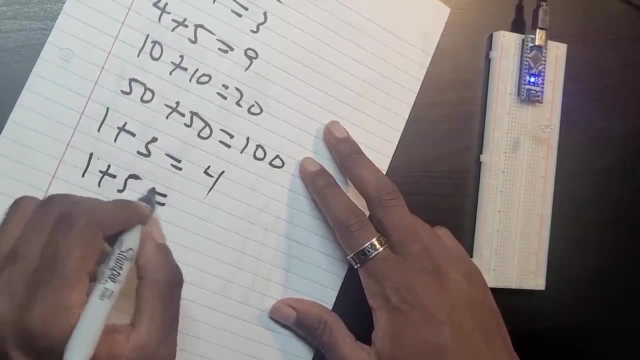 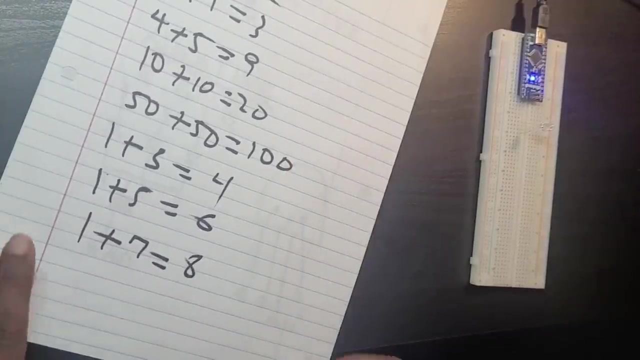 all right, this keeps going. 50 plus 50 is what hundred. okay, and let me just say: one plus three is what four. one plus five is what six. one plus seven is what eight. so the problem is here what let's say. i want to understand how to add up to a million. let's just: 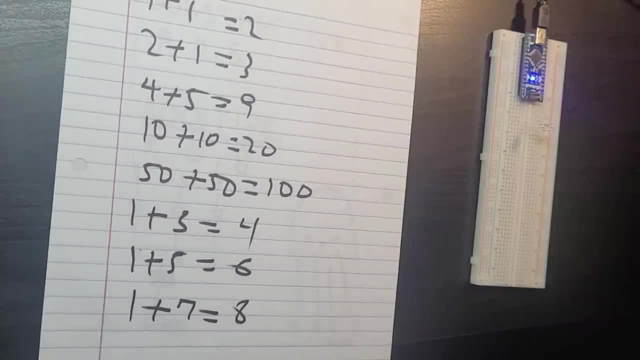 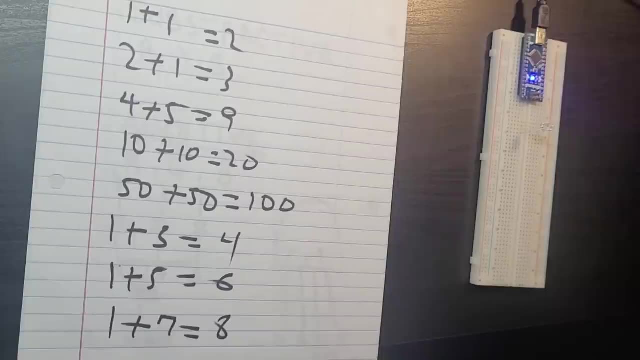 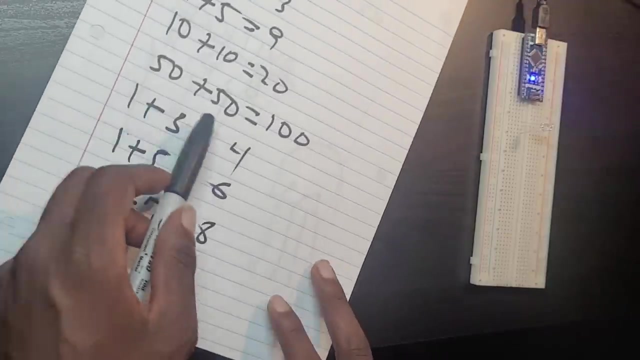 say: i want to know how to even add up to a hundred. let's just say that, all right, i want to catch all the numbers up to 100. let's say: one plus one is, you know, two, okay, two plus one is three. i have to hold what? almost 100 digits to even what, to even count up to 100, okay. but if i learn the basics of 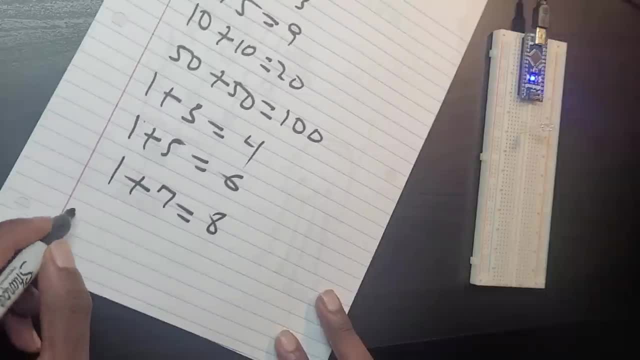 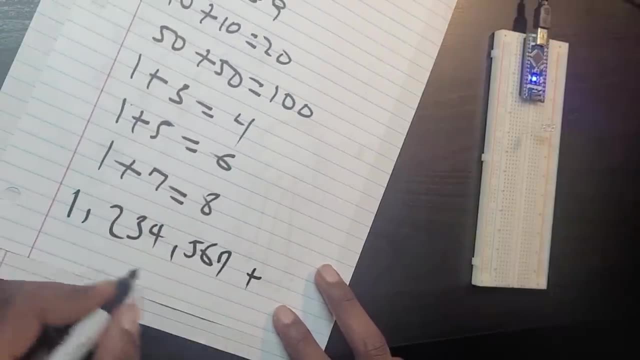 addition, if i learn the basics of addition, i can even add millions of numbers right here: one, two, seven. i can just add this up. it just takes a bit of more time, but i can just technically add it up. i want to add it with one million right here instead of memorizing it. what do i need to do? 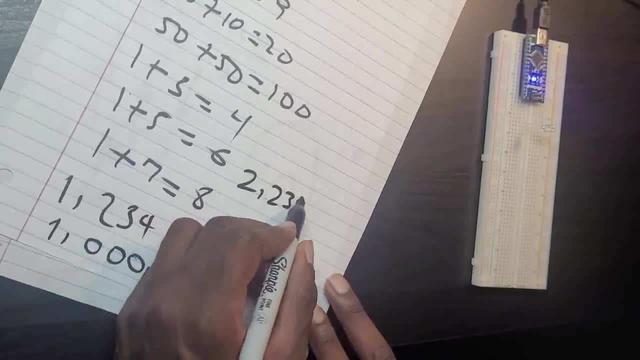 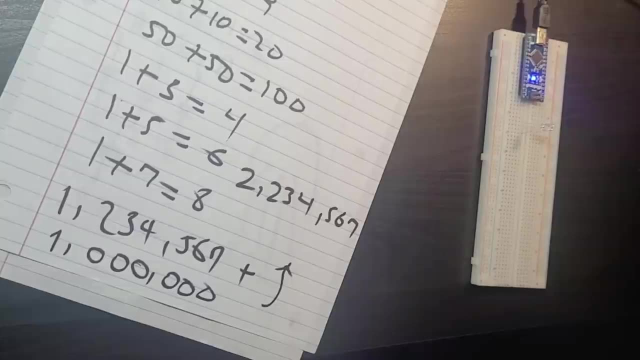 all i need to do is add it up, the answer is going to be two million 234. obviously, five, six, seven. so basically, what mathematics? two is also: what is a system, as you can see right here, and instead of memorizing it, what do we do? we create a system. so, basically, once we create a 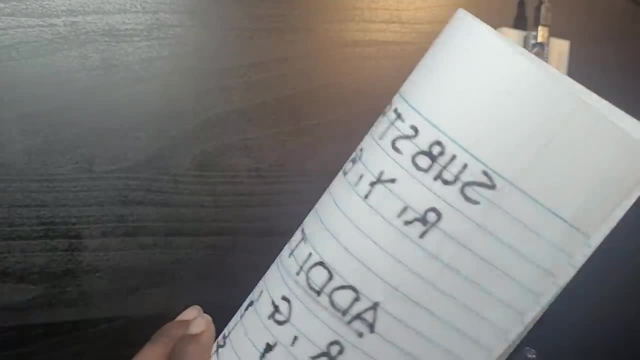 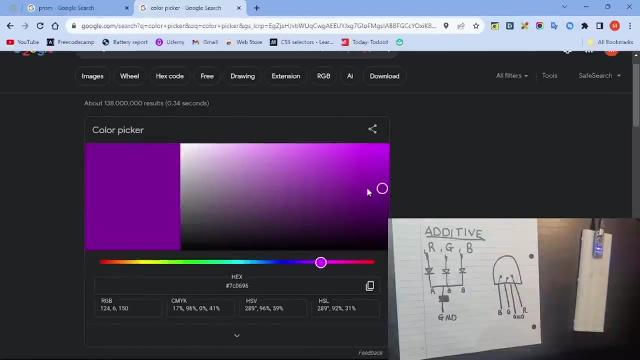 system. it makes what we can count almost infinitely. almost infinitely, as in. you know, obviously we can't count to infinity, but we can do what we can do almost anything. that's why, instead of you know naming it, just think of naming millions upon millions of, again, color combination. okay, just think of naming over millions of millions of color combination. 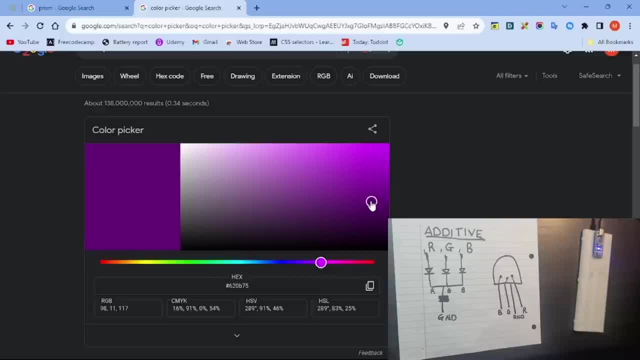 we're going to do is what we're going to create a system of naming it. and then what do we need to do? all we need to do is go to our color picker and then what we can choose: our specific color. you see that right, so we can just think of even. 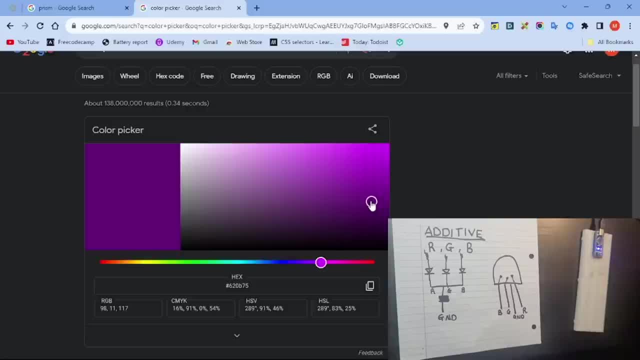 one thousand shades of pink right here. so, like here, let me just go right here. okay, what i'm going to do is move it right here. it's right here, moved, all right, let me just wait. my my. it's glitching out. it's glitching out what happened to my computer. oh jesus, i don't want it to glitch out, all right. 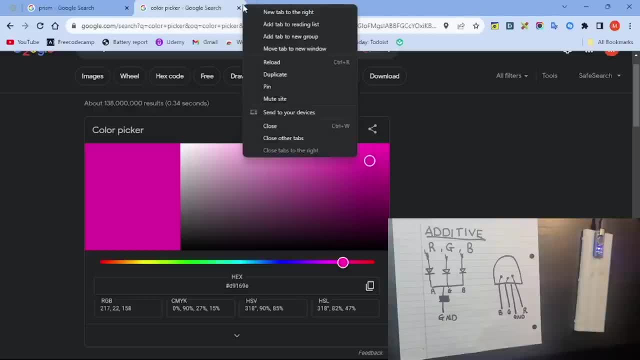 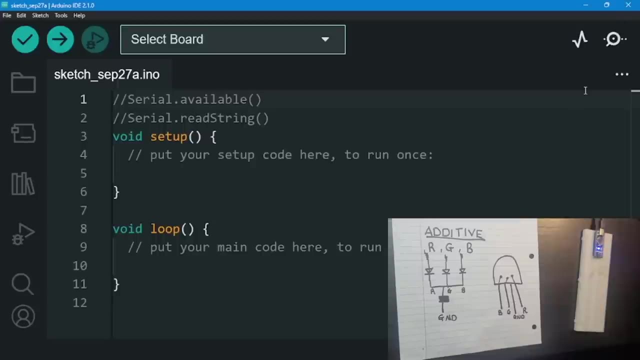 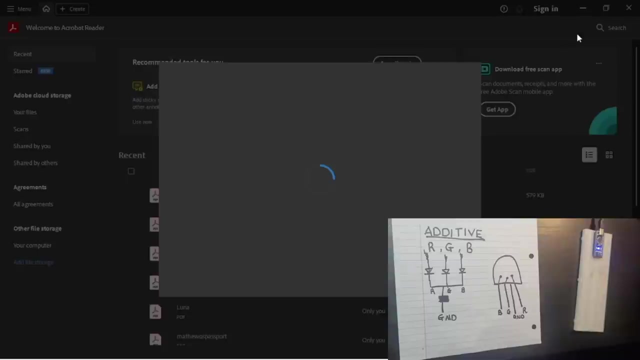 come on, let me just close this tab. what is wrong with it? okay, my, my computer is glitching out for some reason. let me just turn off pro. it just takes a lot upon a lot of uh, okay, come on. okay, it's opening other stuff. oh my god, what's going on? let me just ignore my computer for now. 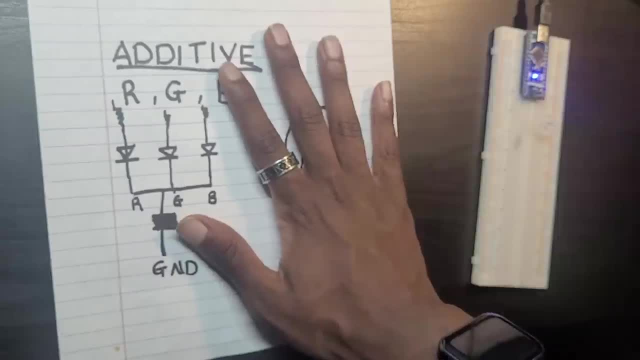 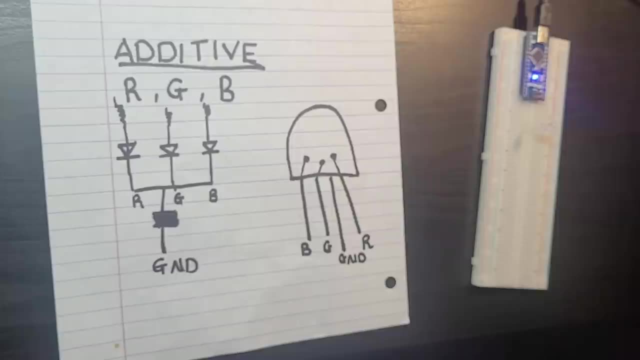 and let me just go over to- uh, let me just go over to this again. so that's why it's very, very important to do what. it's very, very important to have a system of what naming colors, because there's going to be millions upon millions of combinations. okay, 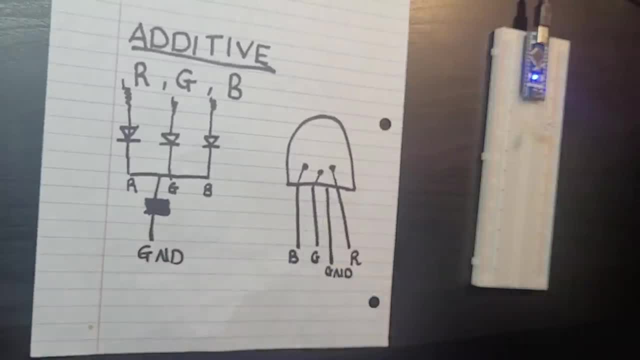 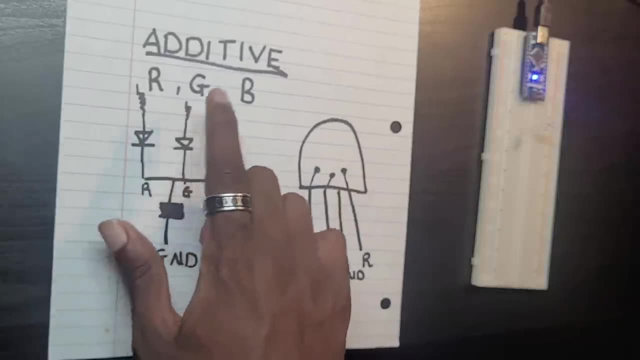 so, with that in mind, we're going to be using one of the most popular naming methods- right, one of the most popular, what color system methods? okay, the color methods, and this one are rgb. there is something else called hexadecimal and i think, uh, some people might know it if you're familiar. 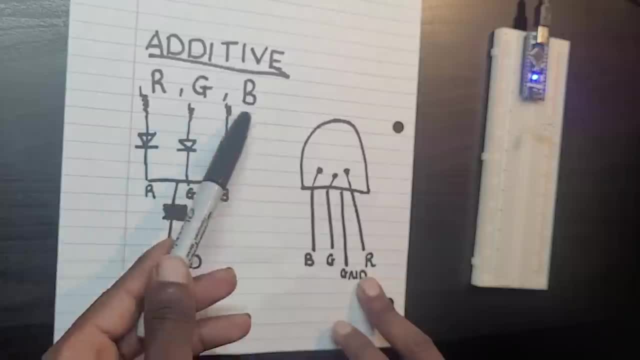 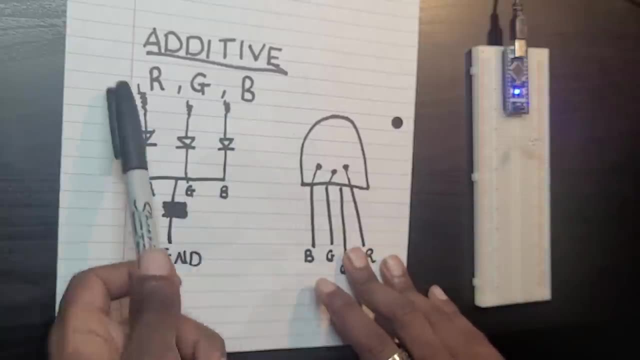 with coding and stuff, but we're going to be using rgb today. okay, because it makes sense, because this is again, as i said, the led is an rgb led, it makes sense for me to obviously talk about rgbs, okay. so now what i'm going to do is: 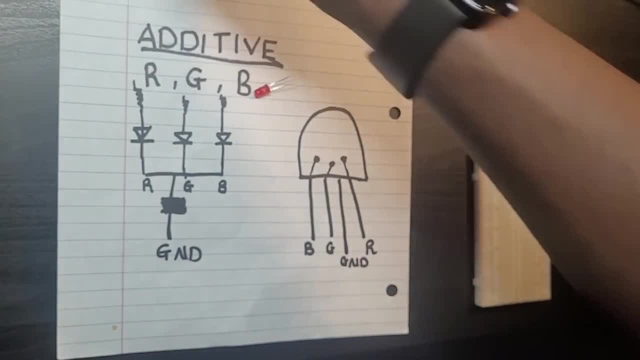 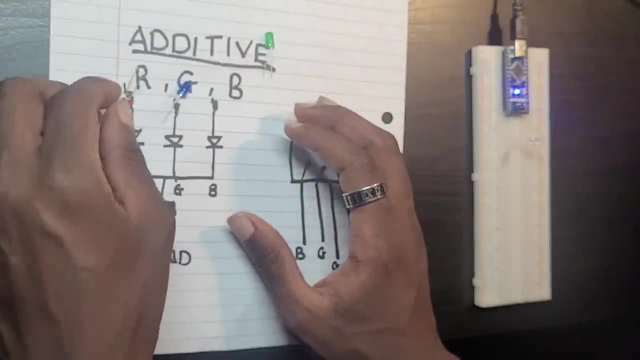 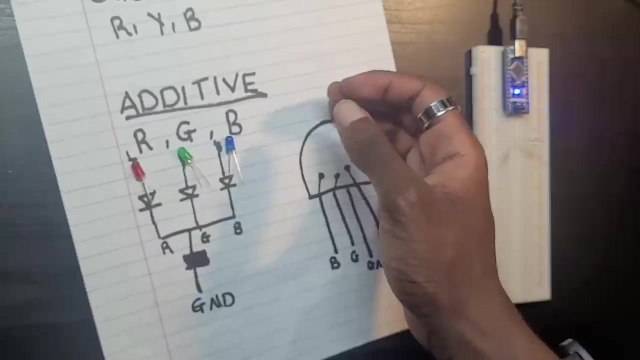 right here. i want you to think of it is as i said again. i want you to think of it as if we're connecting. let me just go put the red right here, the blue on the blue, let me put the red on the red, just put the blue right here and put the green right here and the red right here. so remember. 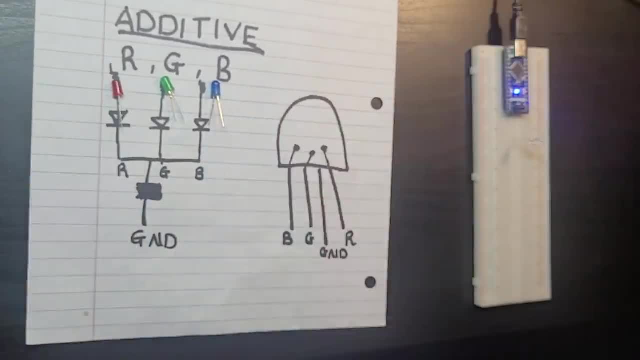 us. uh, oh wait, let's just. let me just put it back here. all right, remember us doing. obviously the traffic light led. what did we do? if you again, i would really be, i would really be appreciative if you just again go back and check it for yourself. 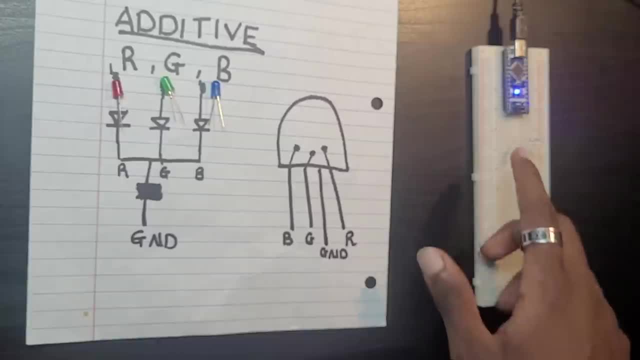 so i'm going to go back to that section and check it. but what we did is what. we connected one resistor to the water- the red, and then what connected to the what, and then we finished, and then we continued to what. we continued to the green and then connected a resistor for itself. 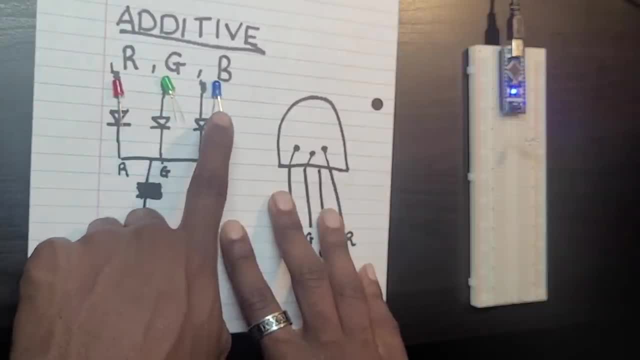 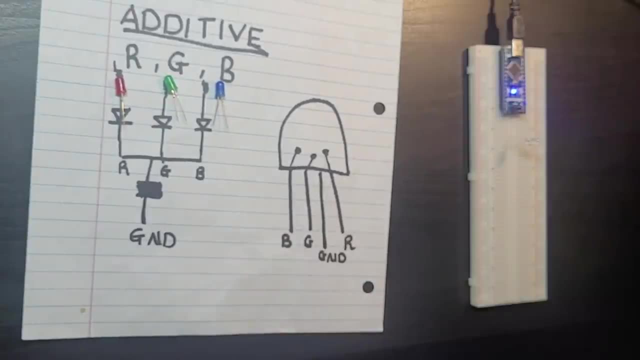 again a resistor for itself, and then we connected another resistor for what? for blue? and then we did what. we finally connected it to the gnd. that's what we basically did. so one thing i want you guys to keep in mind is: just because it's just one led, don't think that's. 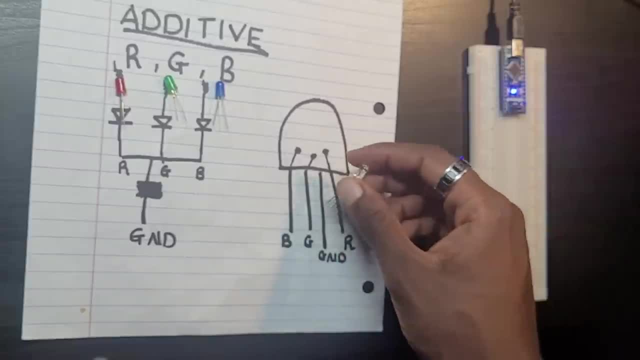 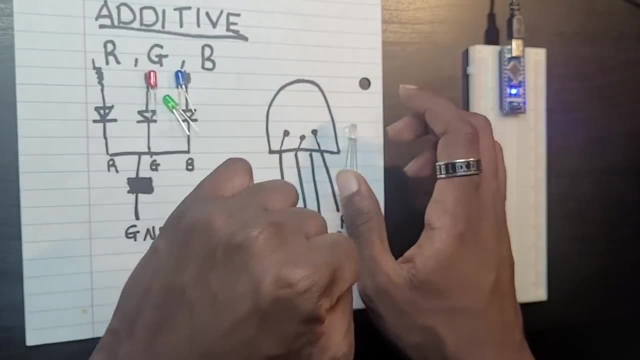 just one led. we need to wait. so what we did, we have to, what we have to, use only one resistor. all right, i just, i just told you guys, i want you to think of what i want you to think of: just us mashing up this three leds, these three leds into one. okay, just think of mashing of these. 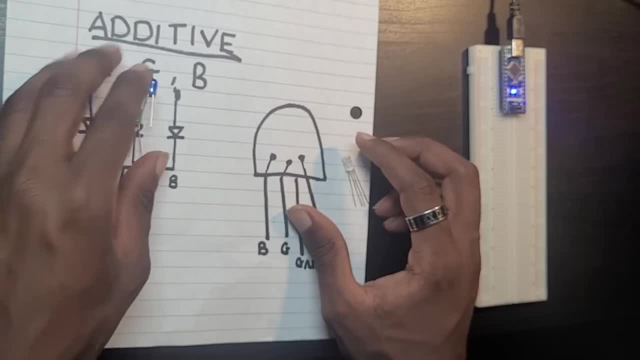 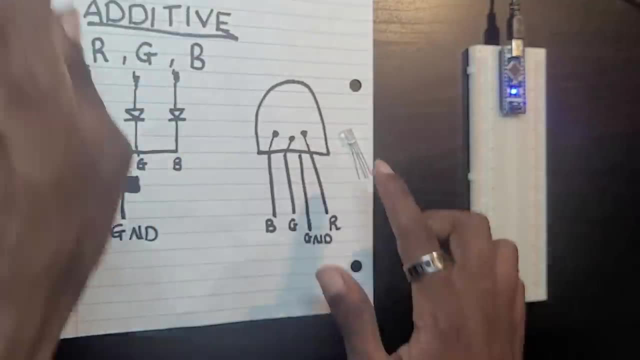 three leds into one, then having a fourth leg right here for gnd. that's all, i think, what you guys, we did, right. so just think of mashing up again. what did we do with this RGB LED? just mashing it up together. so we're gonna need three resistors here. i want you to keep that. 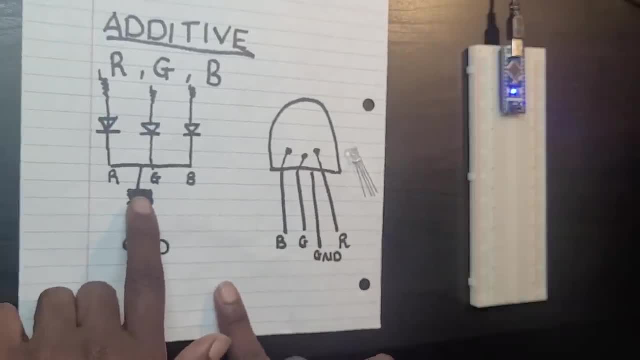 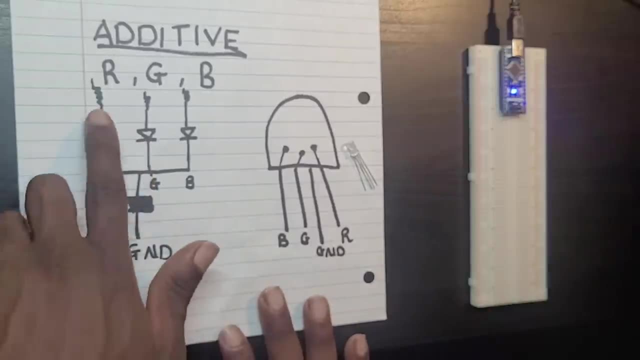 green and blue. so, right here, don't use one resistor. i think this is something that, uh, a common mistake that happens, so please prevent that. so again, always what? use three resistors, because we're gonna be what lighting up red, green and blue. i just like, as i, as i said again just: 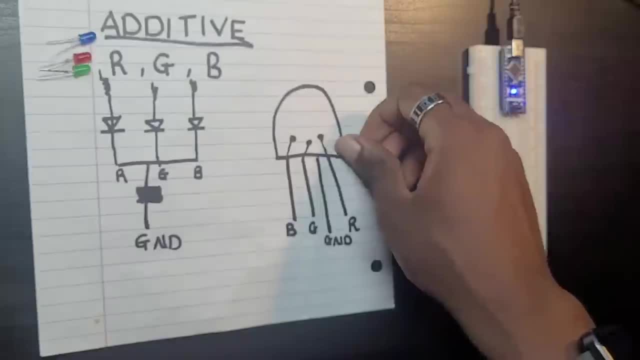 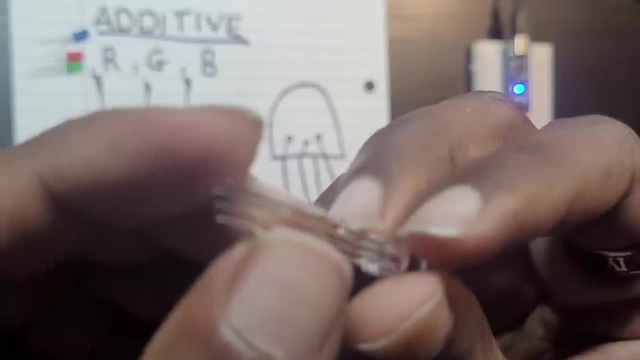 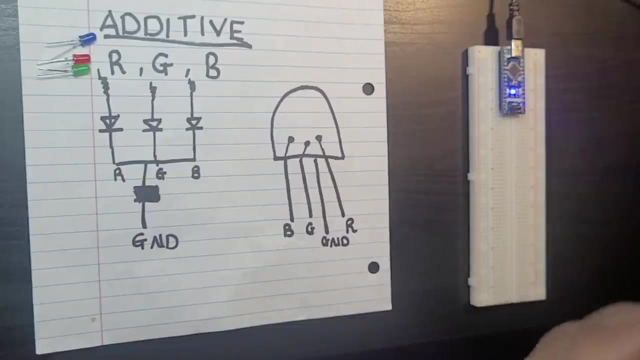 think of it as what? as three mashed up resistors. okay, so as three mashed up what leds, okay. so let me have to put this back again. i have to find the longer side again, which is a bit of a hustle. oh, it's actually a bit hard. oh, i found it all right. there we go. it's like this the longest. 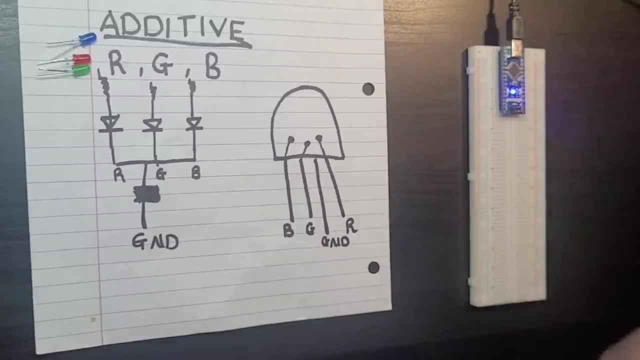 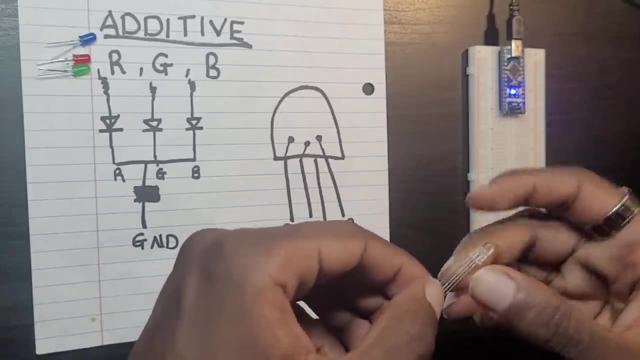 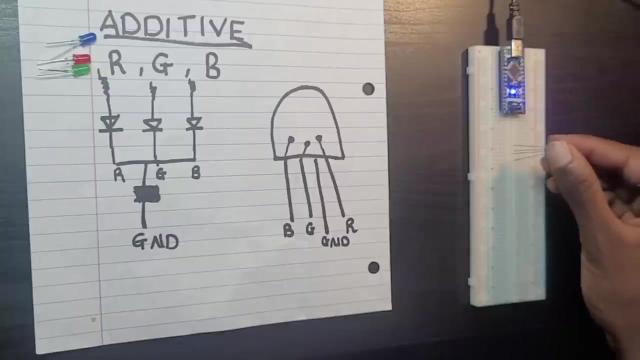 side is obviously the ground pin, where the ground pin goes. so let's start working with our led. now is the right time, i think, to work with our leds. i have to widen this a bit again. i have to widen it so that it goes across, to push it a bit. there we go, all right. 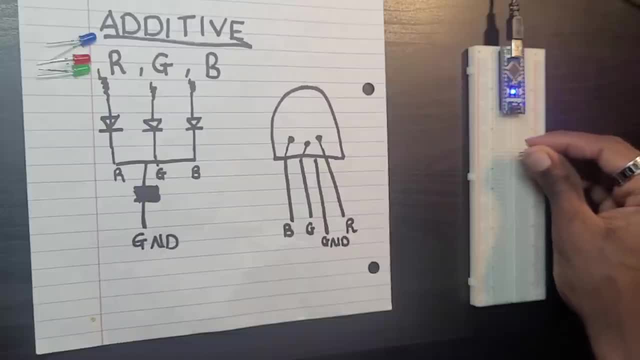 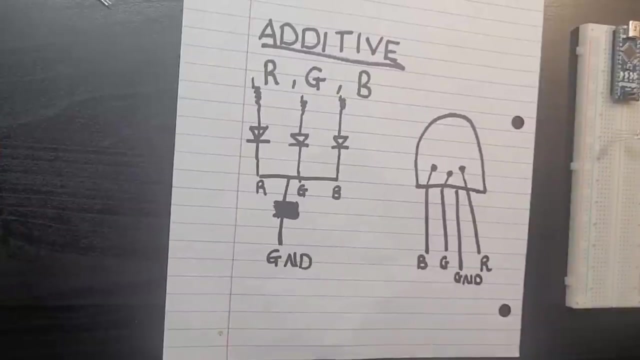 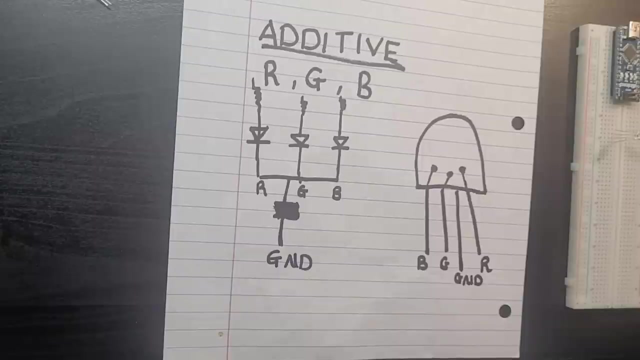 come on, okay, come on, come on, there we go. got it, okay. so let me just go back to my pc. hopefully, okay. for some reason it's glitching out, okay, so sorry, my computer just crashed, but uh, let's continue where we left off. so, as i said, 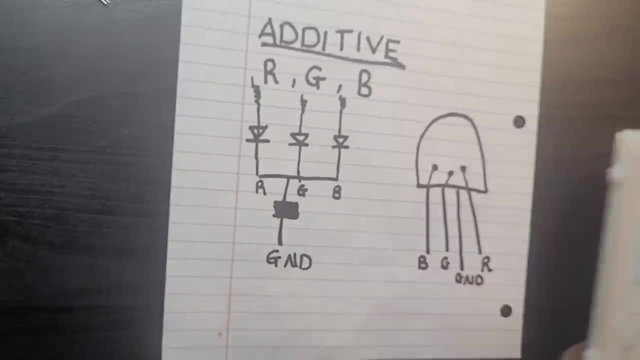 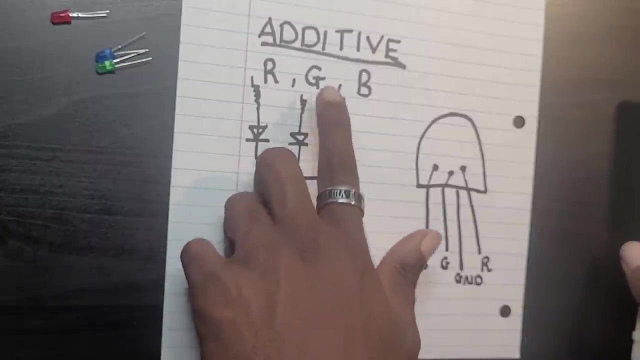 again. i just want you to think of the rgb led as what, as three leds, separate leds, what combined into one? okay, that's what i just said. obviously, it's going to be very similar to the one that we just did to the uh traffic light. of course, but instead of using green and, sorry, instead of using yellow. 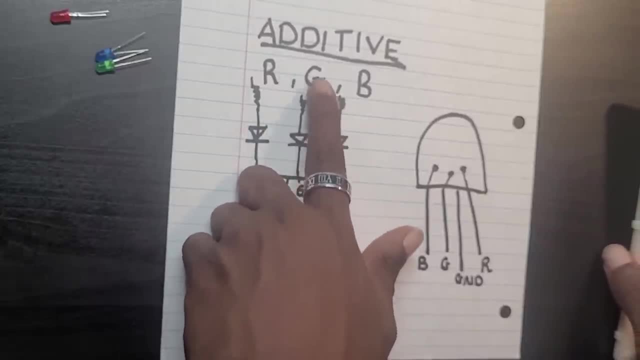 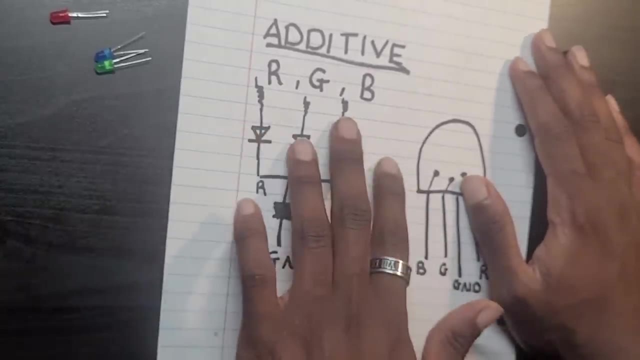 we're going to use what green here, okay. so what did we do in the traffic light? we separately did what again? we separately what connected three digital pins, three resistors, and then connected it. so what we're going to do right now is going to set up what? three again digital pins for each. 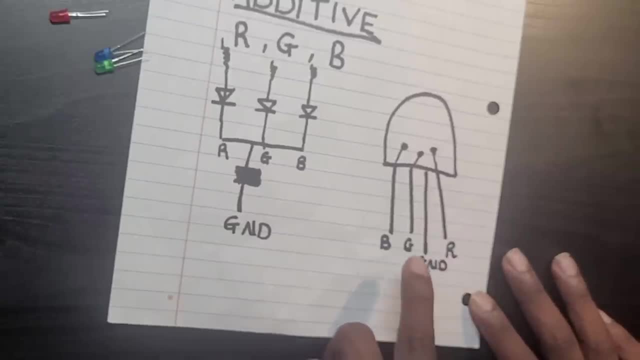 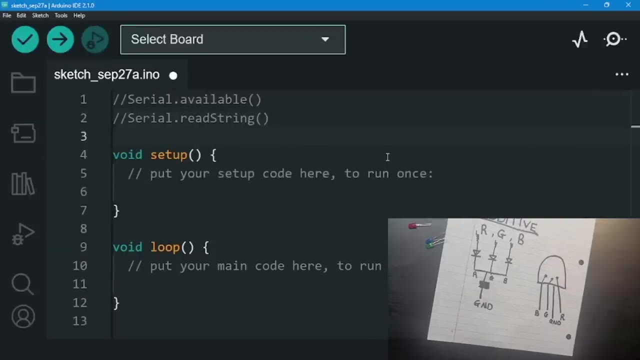 color. so we're going to be setting up the leds and then we're going to set up the rgb leds, one digital before red, one digital bit for green and one digital pin- for what? for blue? okay, so let's just do that. okay, forget about the comment, the comment that i have here. 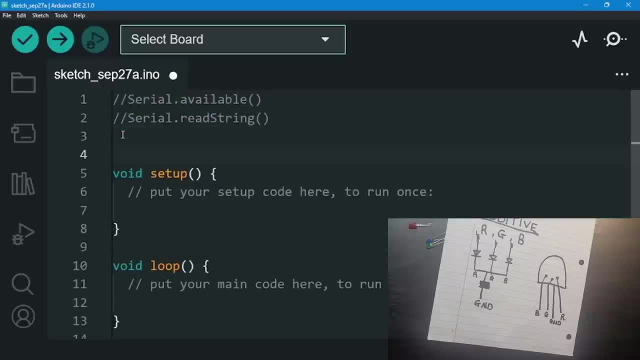 okay, i'm just going to get back to this. i just want to remind myself to teach about this along the way. so we're going to get back to this, but right now i want you to focus on what we're going to be creating: three digital pins. so it's going to be red pin. right here we're going to start with. 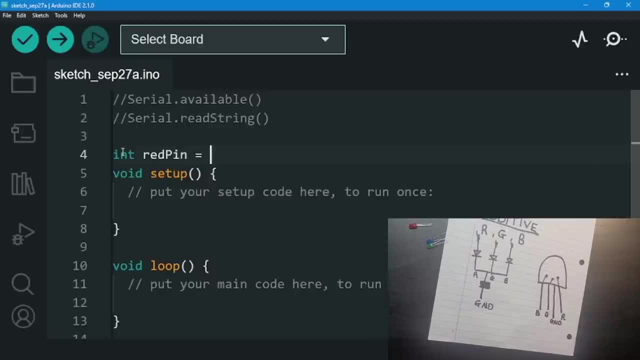 red pin. i'm just going to set it up to one digital pin. i'm just going to say four today. again, you can do whatever you want to int. then i'm going to choose the green pin. what is it going to be? again, five, eight, any number you like, i'm just going to press five. i'm just going to try to make it. 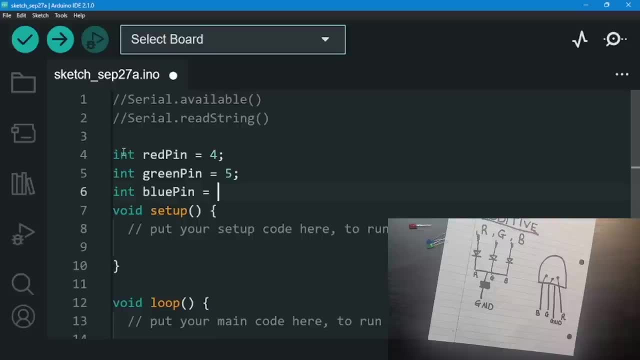 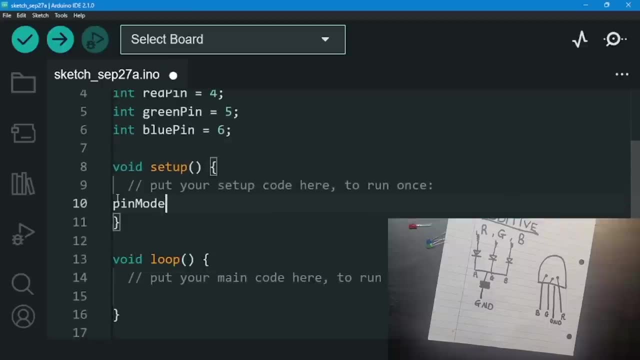 consecutive, and then we're going to go to blue pin and set it to six. all right, then afterwards, what do i need to do? i need to go to pin mode, then set it up to what i need to go to pin mode, say red pin in this case, and set it as what output. 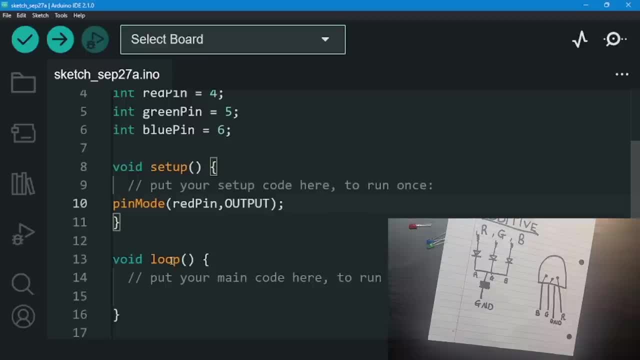 once i'm done with that, obviously, what i have to do is copy it. so to do this in an easier way, what i'm going to use is a shortcut alternate shift and then point downwards. i'm going to be using ultimate shift, holding it together, then i'm going to point downwards so i can copy it again. see it. 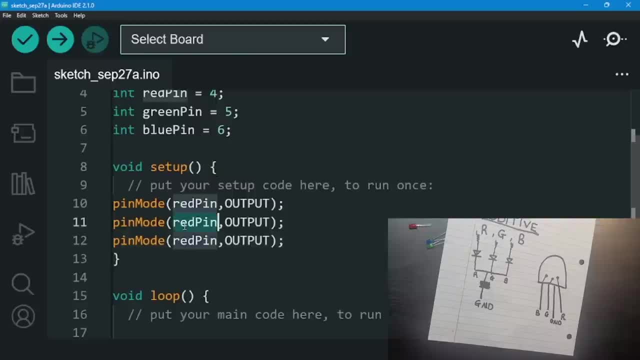 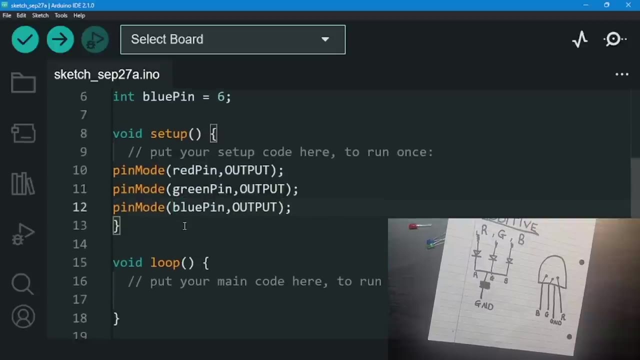 i'm going to copy it three times then. now what i have to do is what? change the pin right here. i just changed my language. let me just change it back to english. there we go, set it to green, pin this to a blue thing. all right, then afterwards, what do i need to do? as always, i need to what i 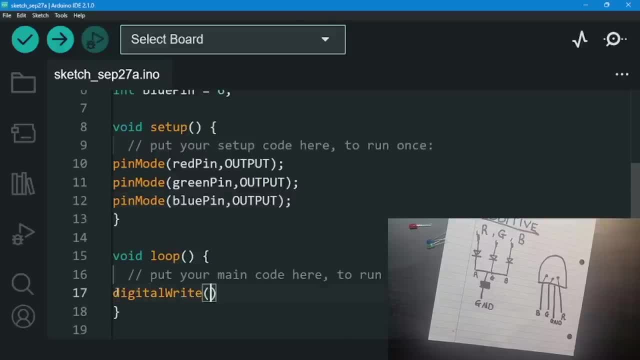 need to use digital right, because i'm working with a what with digital pin, then i'm going to say red pin and set it to what? to the value of high. all right, again use alternate shift and again click down because again, as i said, again, it's going to make things easier than copy pasting. 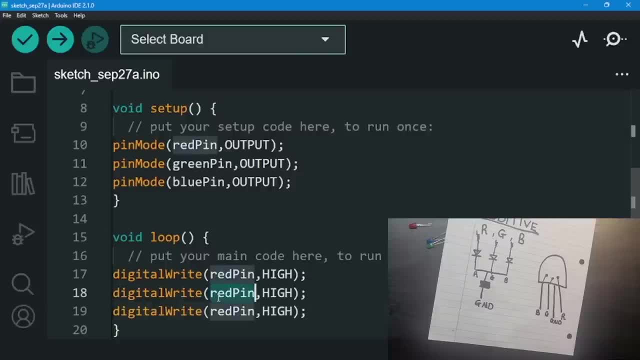 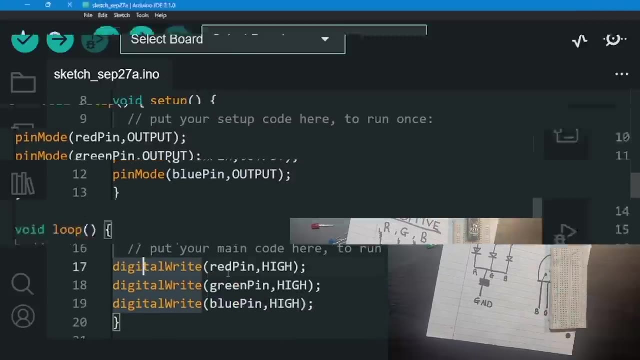 them, writing them from scratch. so all i need to do right here is what? change this to green pin. and then, what do i need to change this to? i need to change this to blue pin. all right, so we're done. uh, setting up the code. so let's start working with our components. okay, so let me just get this. 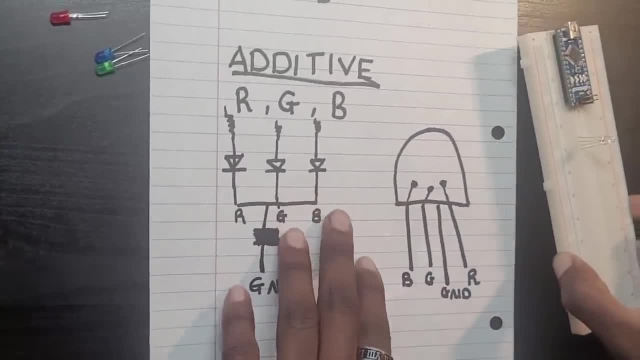 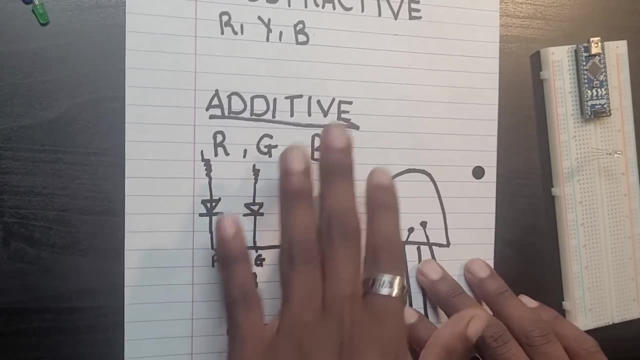 out of the way. actually, i should let us stay here, to be honest, because it's a bit of a harder concept, so i wanted to stay here. so again, you guys can reference this. all you need to focus on the subtractive, let's focus on the additive and again, these three things. all right, just want to focus. 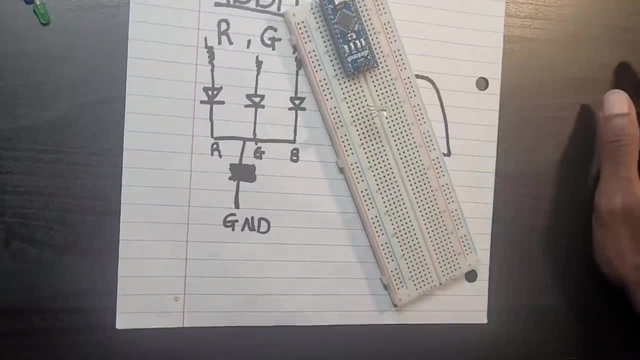 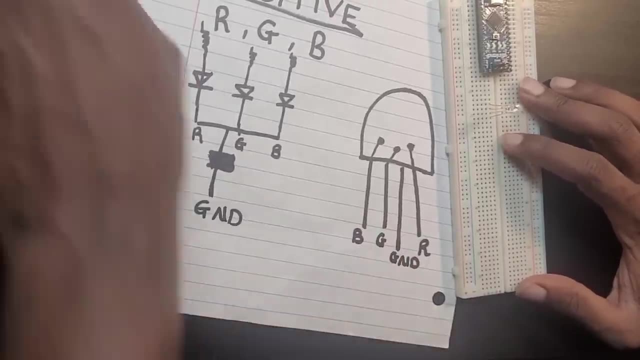 on these two things, okay. so what i'm going to do right here is i'm going to be using the red one for the red. right here, the red is at the fourth. the green one. the green one. i'm going to be using a green wire. for what? 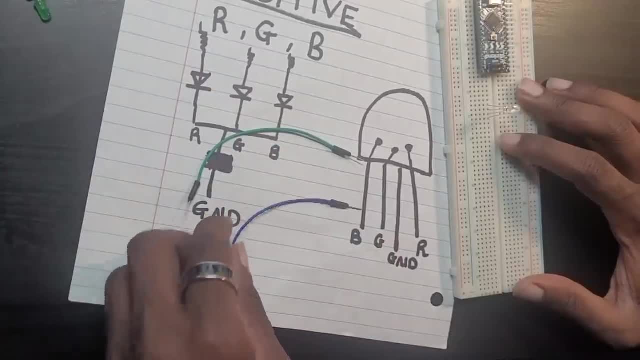 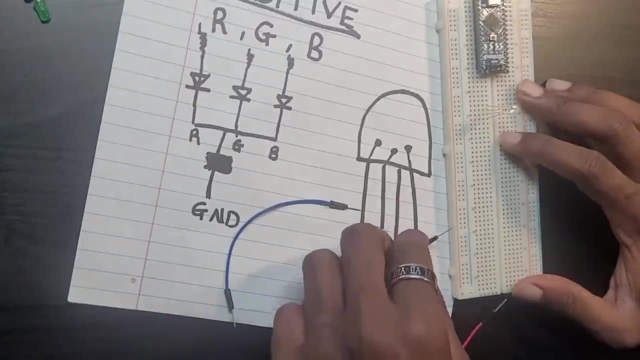 for green? a blue wire for what? for the blue color? that's what i'm going to be doing: green, blue here, green here and the red here. that's what i'm going to do, and i'm obviously going to use the gnd. for the gnd i'm going to use. what a black wire? okay, so let's just do that. 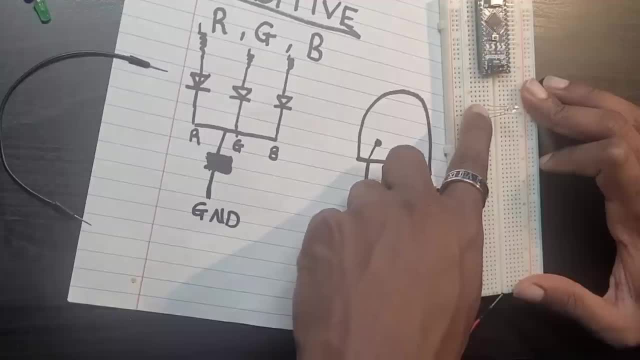 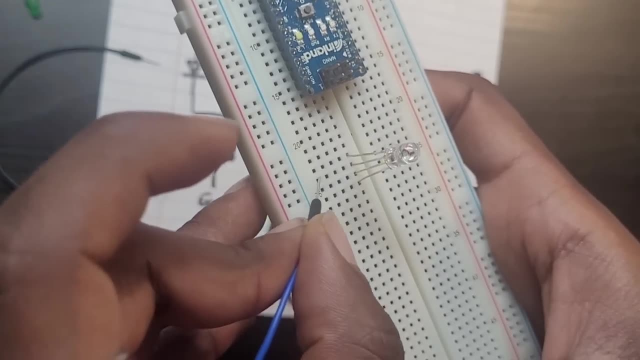 so let me start with the blue one. it's going to be the one at the very most left, so let me just connect it. let me get this closer and let me connect it. let it focus now. let me connect it. there we go. then, what am i going to do? right here, i'm going. 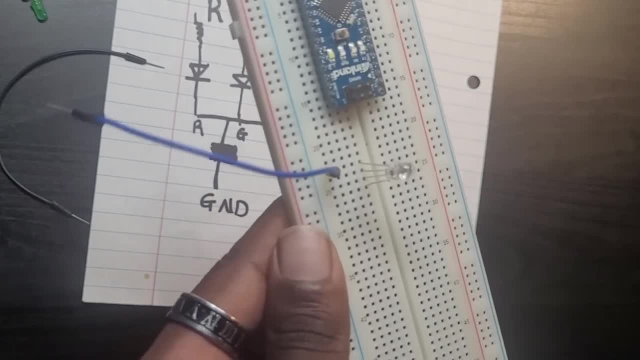 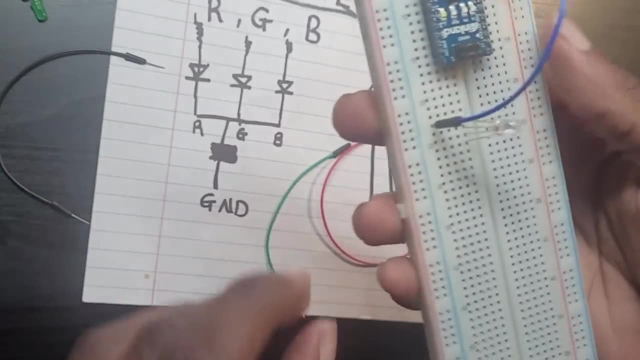 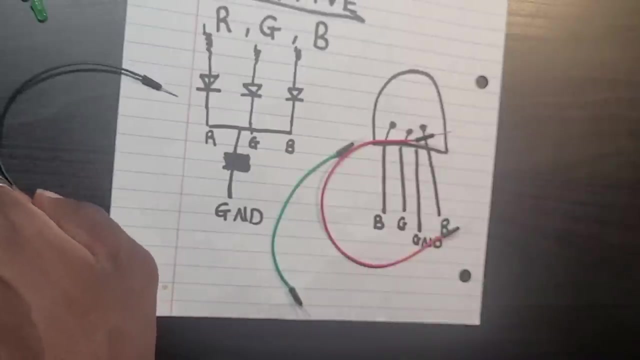 to be connecting it to pin what again? let me pin it's pin number six. okay, pin number six for me, pin number six. there we go. then i'm gonna connect the green one, let's just do that. i'm just gonna go ahead and connect the gray one, then i'm going to control the recorded one. 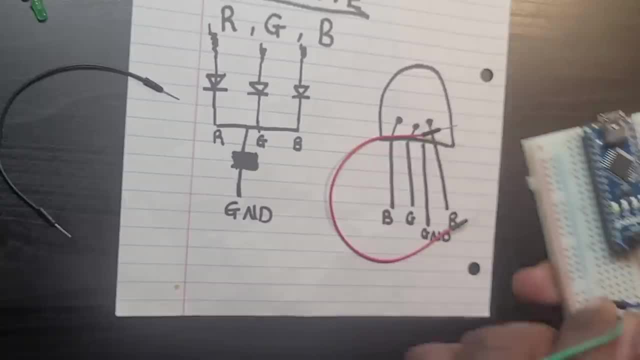 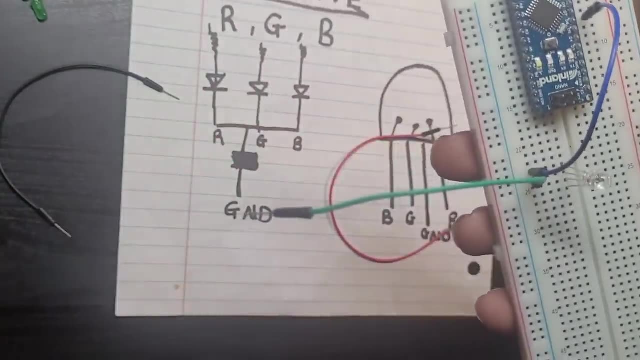 right here. let me change the green one to the upshot one. oh, i can do that now. oh, let me connect the green one now. rất cool, okay. so i'm going to do this for the green one. just connect the green one with what? with the green wire. so let's go to the green one right here. 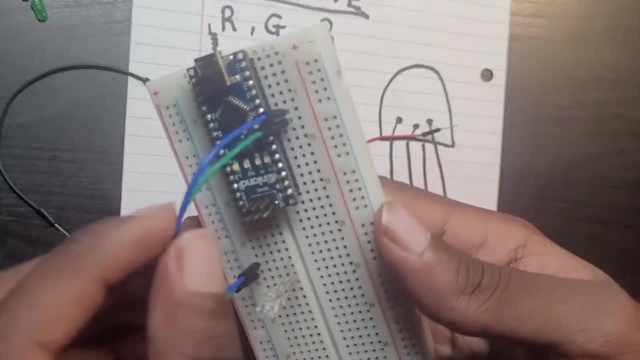 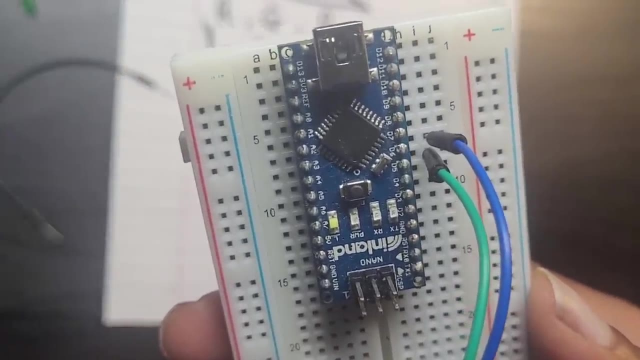 this is going to be next to the blue one. there we go again. make sure that you guys can actually see it. focus here. there's still pin five, hopefully. focus there we go now you can see it, there we go. there's still pin what connected. there's still pin six and 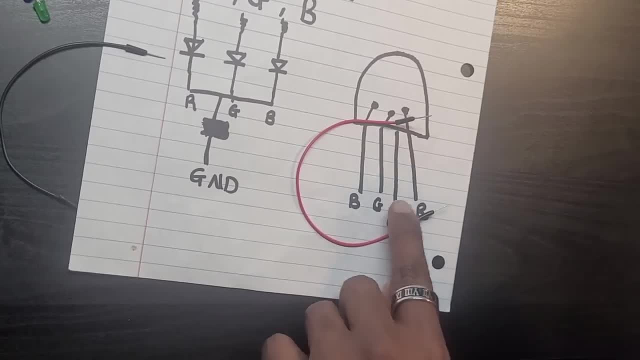 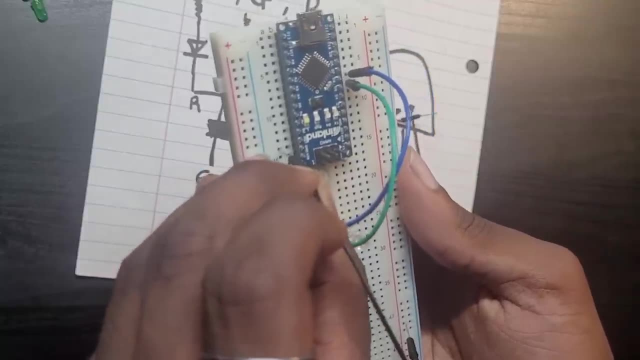 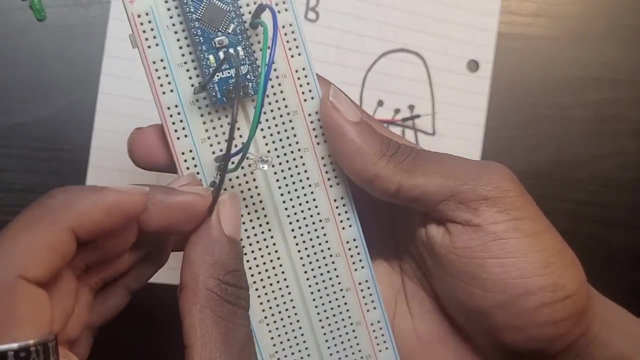 then there's still pin five. now the one that is left is what? gnd? okay, let me bring my black wire right here. let's get my black wire and let me connect the gnd. there we go, as you can see, connected to the gnd, and then now i'm going to connect it to the third, to the third leg. 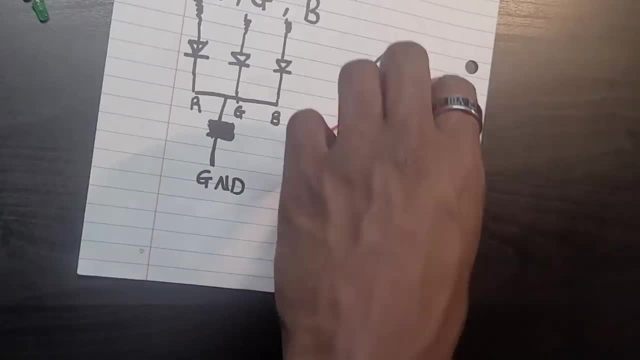 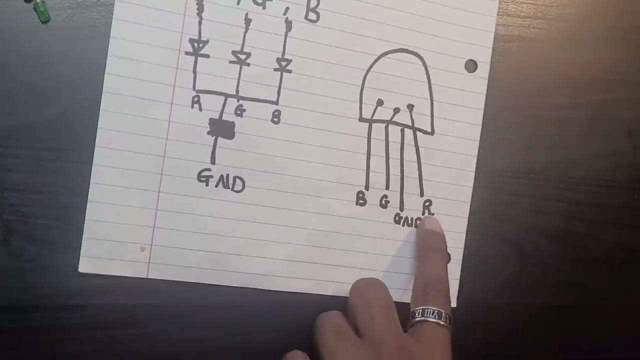 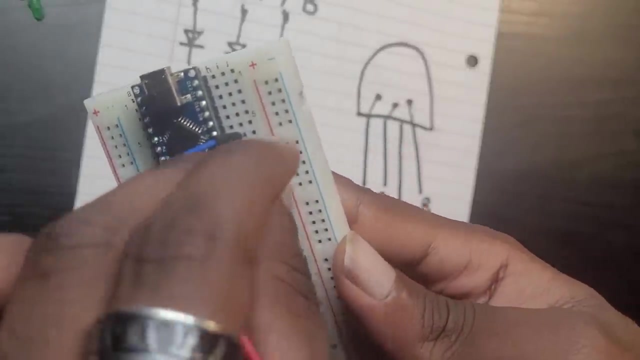 there we go. third leg connected. all right, then, now the fourth one i'm going to be connecting with what? i'm going to be connecting it to the red. so the red pin is what it is. pin four, so additional pin four, let me go to digital pin four. just did that, let me just do that. so let me just focus. so 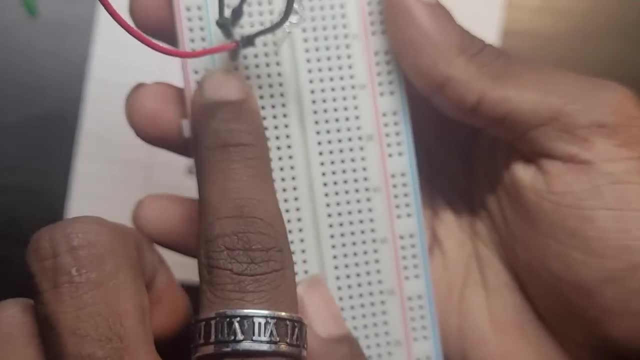 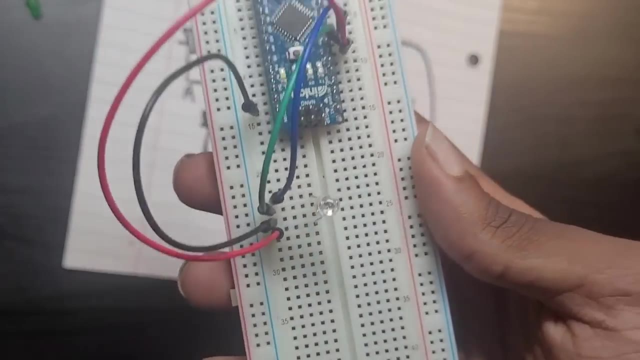 you can actually see it. i connected the digital pin four, the which leg, the fourth leg. there we go, focus it right here. the digital pin, what digital pin four? all right now, i can just what i can just run, so all i need to do is upload it. let me connect my. 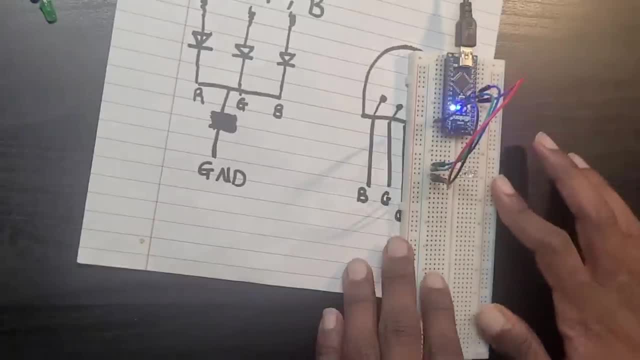 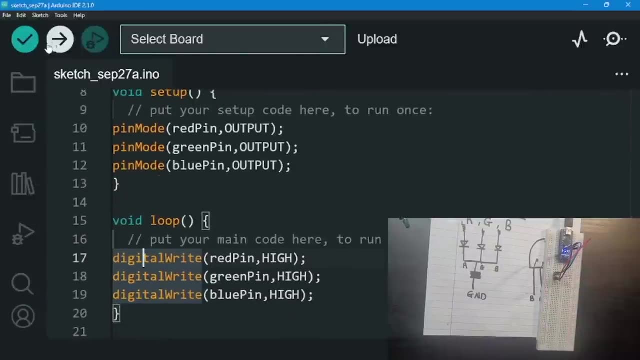 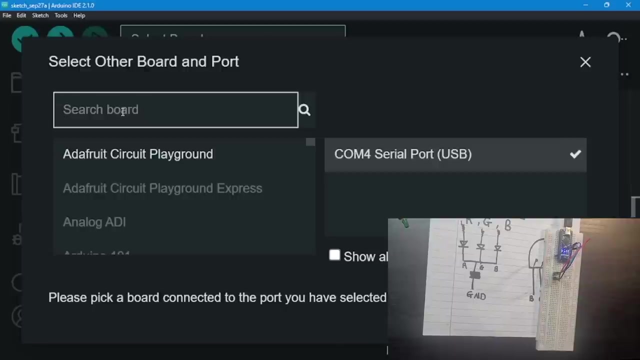 arduino. let me just plug in my arduino right here, right now. i can just run it, so let me upload it. all i need to do is verify the code. is this new board selected? let me select. my board is unknown. let me select that again. sometimes this happens i'll have to say it's arduino nano. 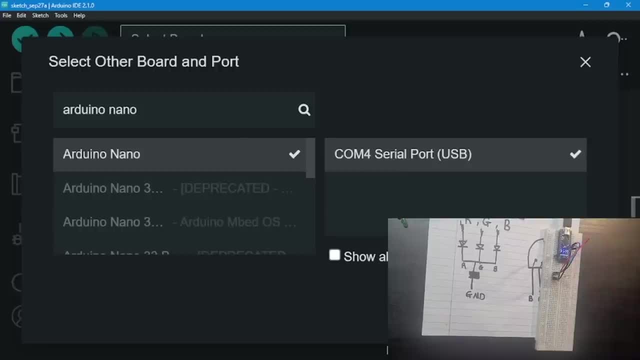 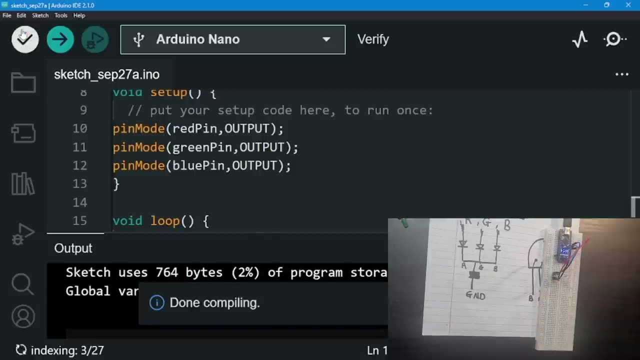 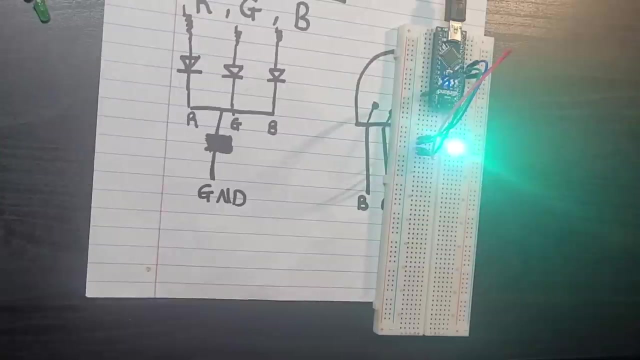 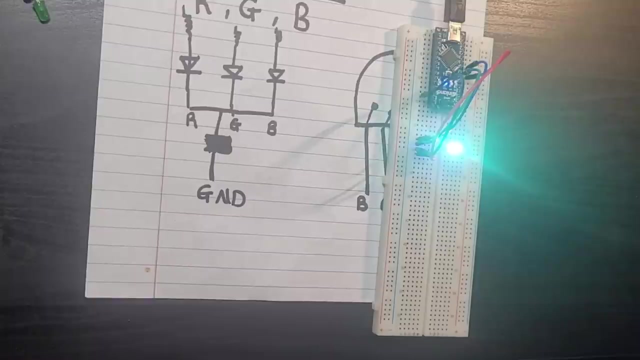 there we go, got my com4 serial port. there we go. and now we should be, should be able to verify, and it's done compiling. now let's upload it, okay. so let me just turn off the light so you can see way, way better. let me just do that because it looks like a greenish type of light right now. 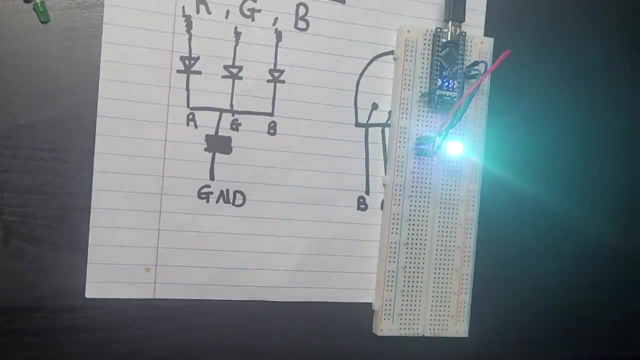 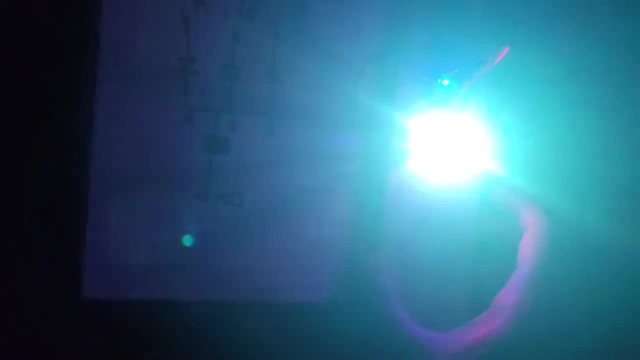 let me just turn off the light here. both lights actually just turn this off too, so you can actually see it. it's too bright right now. let me just try to focus it here. it's a very, very bright light. you cannot, but you can barely see it. 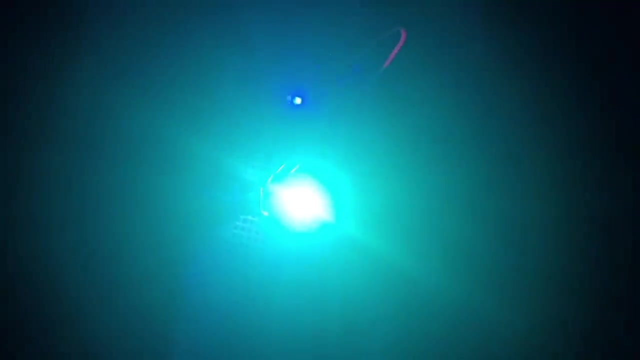 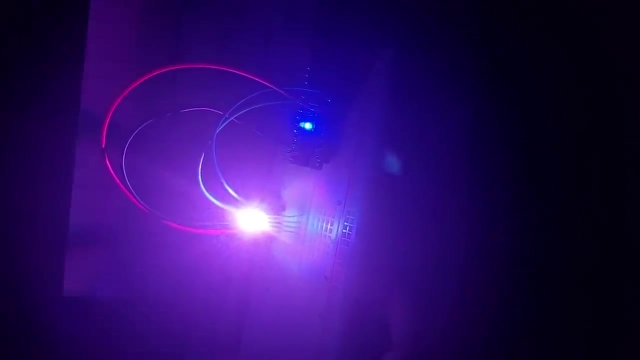 it's trying to give me. can you see green? sometimes you can see red, mostly you can see green. but let me go over to this direction. it's really hard to actually get a lock of this, but it looks somewhat like what somewhat like white, okay, somewhat like what somewhat like white whitish. 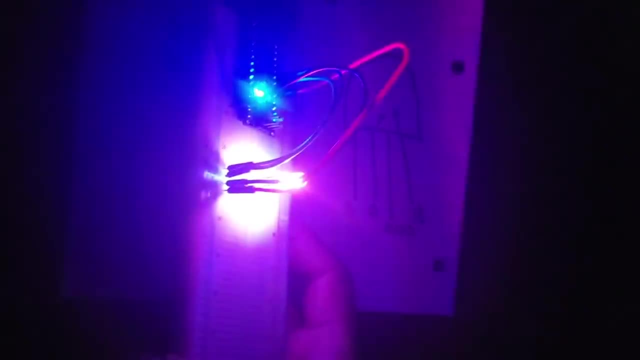 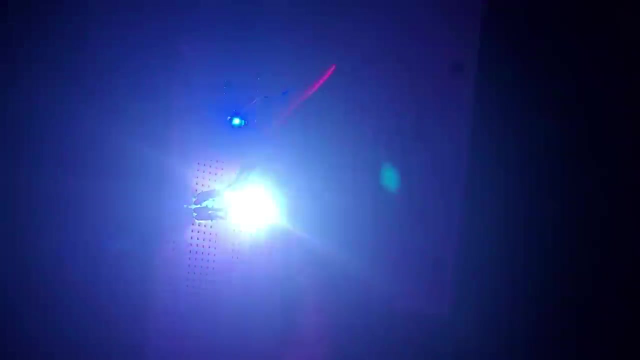 type of color, but when you put it here, when you look at it on the screen, it looks like green. but genuinely, what i'm getting is what i'm getting- uh, white light right here. by the way, i'm, i can look at it. white light somewhat looks like green on the screen right here. can you see it? you can. 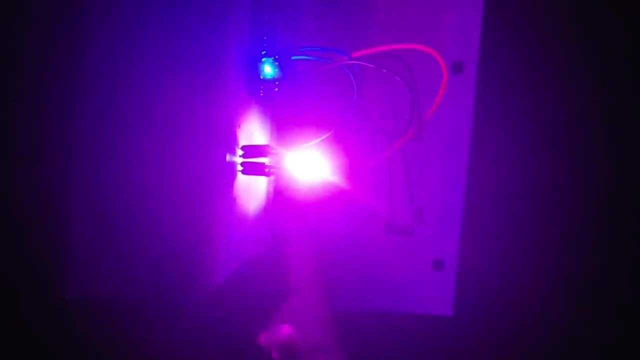 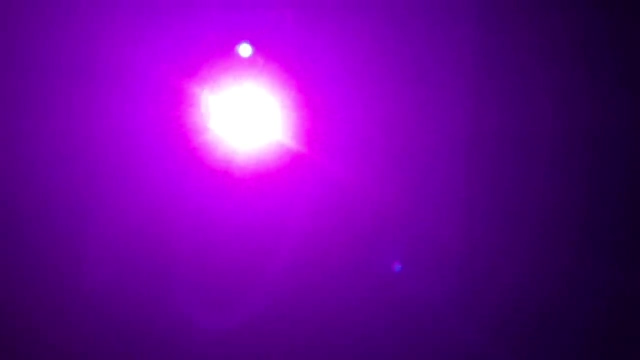 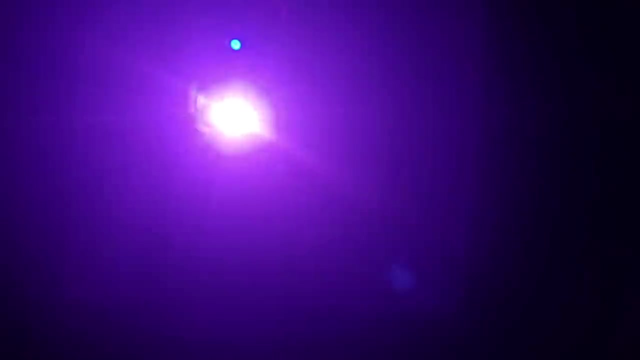 see dynamic range of what colors right here. i can see a red right now. can't you see a red right now? can you see we have red, green and blue. when we combine them, it looks like somewhat like what? somewhat like white. so one thing i did not do right here is what, by the way, one thing i did, 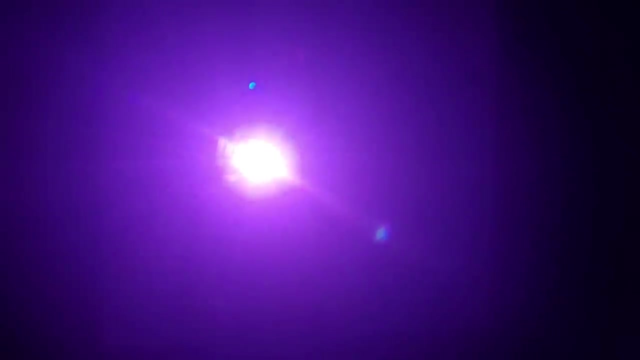 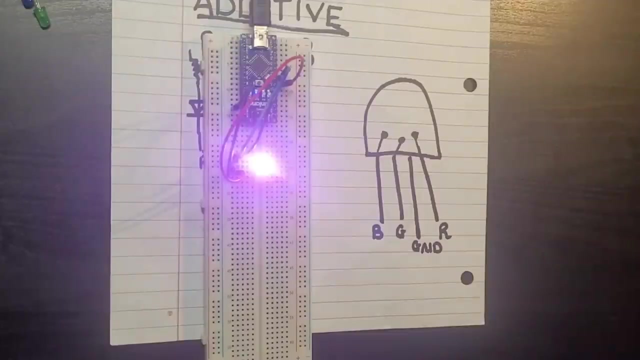 not do right here is what use resistors? i want you guys to keep it in mind. i did not use a resistor. well, specifically speaking, right here, you don't have to use a resistor. right again, specifically speaking, you don't have to. what use a resistor? but? 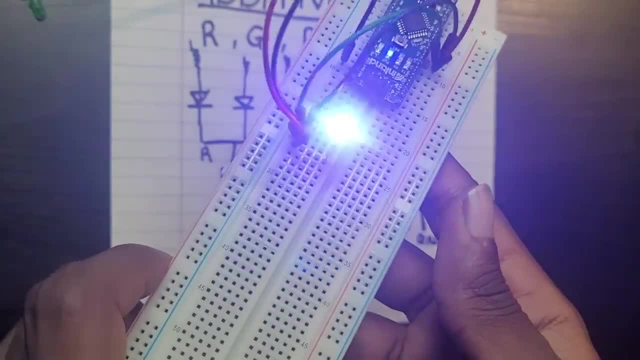 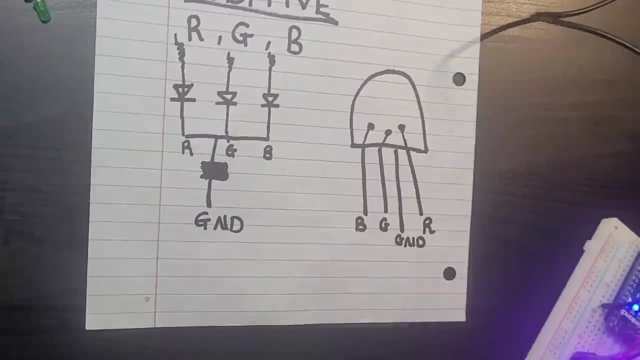 it's not really stable. when you look at it, it just looks like it's changing color every time. by the way, it's not. what is happening is what. there's a red one, the green and the blue are lighting up, and when the camera focuses, it focuses only on one color. you get me right. so when i 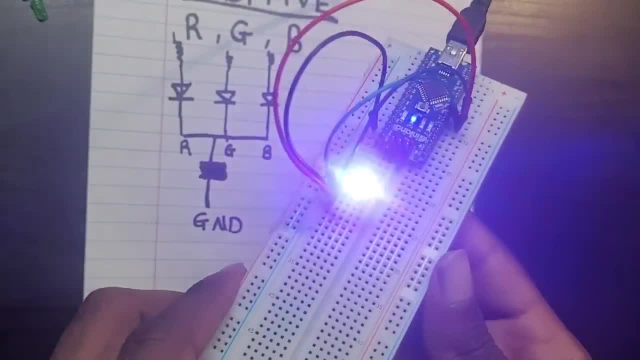 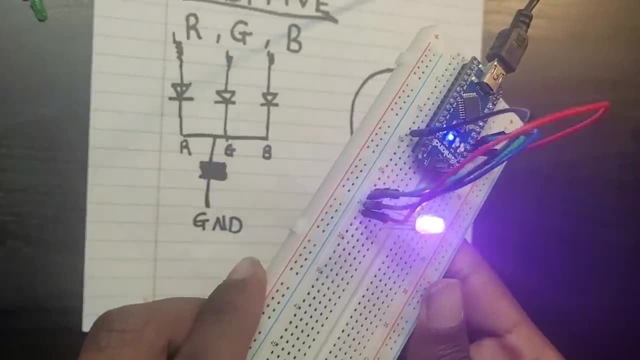 change it right here, it looks like a reddish. when i change it a bit to another angle, can you see it? you can get a bluer, greenish thingy. then when i change an angle again it renders it as another color. but generally what i can see is what? mostly what i can see is white, but if you look close, 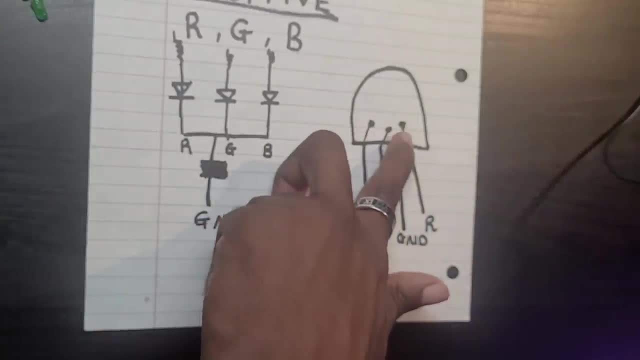 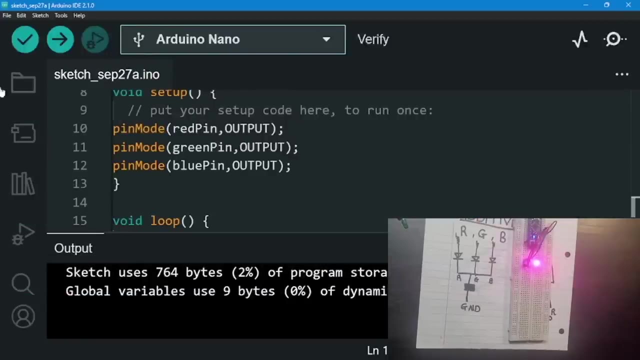 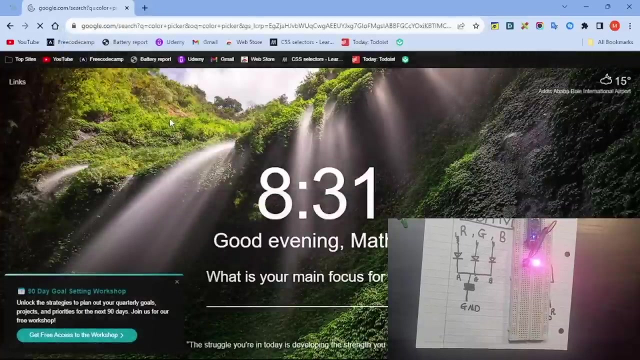 enough. you can see red, green and blue. those red, green and blue are turned on. okay, okay. so let's just keep that in mind. so if we go to my screen again right here and let's go to our color picker, let's do that. i have to google it again because i just said again, my computer crashed. 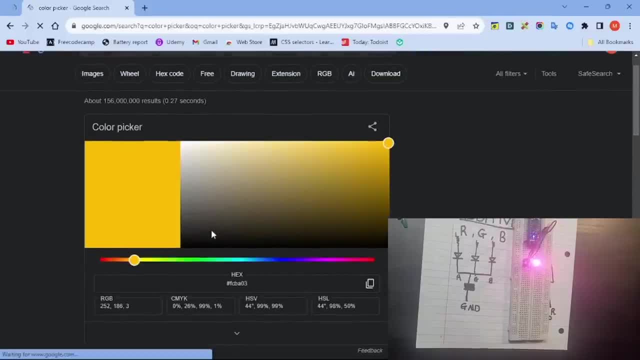 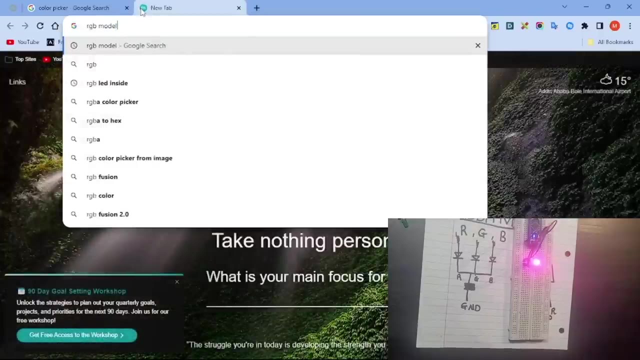 color picker. and if you go right here to the very most white, it is what it's: 250, 250, 255,, 255,, 255.. Basically, it's turned on to its maximum and maximum and maximum. Even if you go right here and say the RGB model, just say the RGB model, and then you 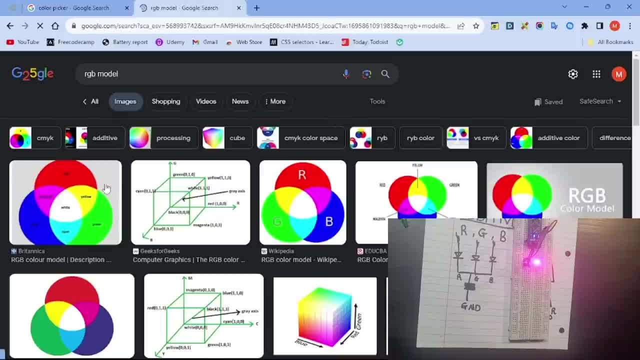 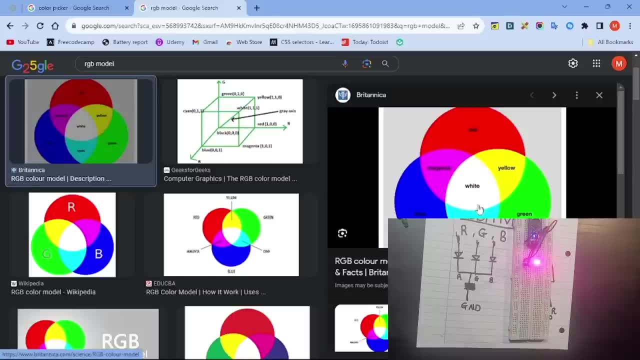 Google it. if you look at it, the intersection of the red, green and blue, the intersection of all of them, is what It's white. When we turn all of them, what happens? It turns to what It turns to white. 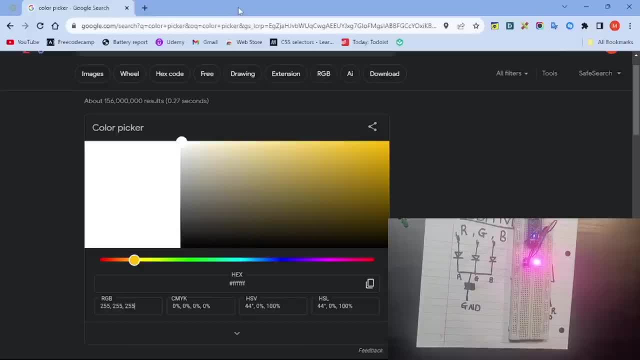 Okay, So the intersection of all is what It's: white, Okay. So let's just get this in mind. Okay, So one thing again we've worked with. let me again familiarize RGB for you guys. We actually did what? 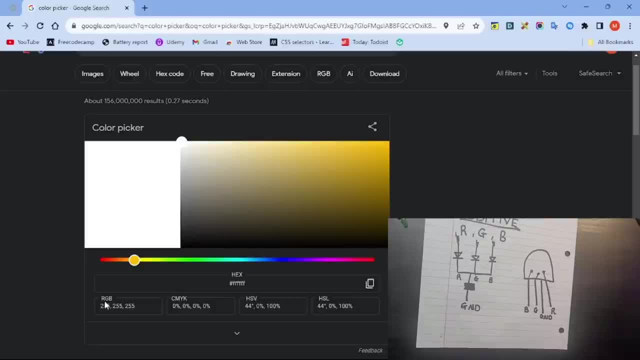 We actually turned on all of this. It's beautiful. Let me just bring a paper right here and let's go to the math side of it. As I said again, there's going to be what A math side towards it. 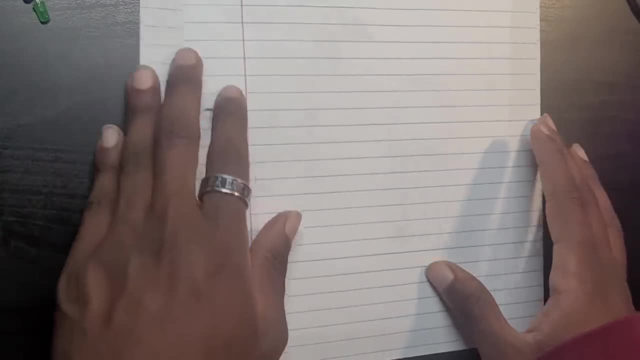 That's like how we again use math to again systematically what Add and all, instead of what Memorizing We're going to have this involves. This involves a bit of what This involves a bit of numbers, Okay. 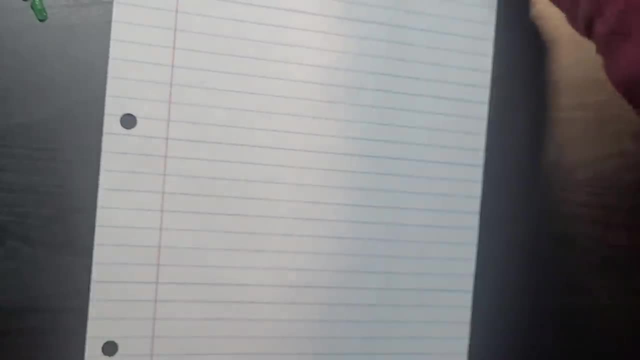 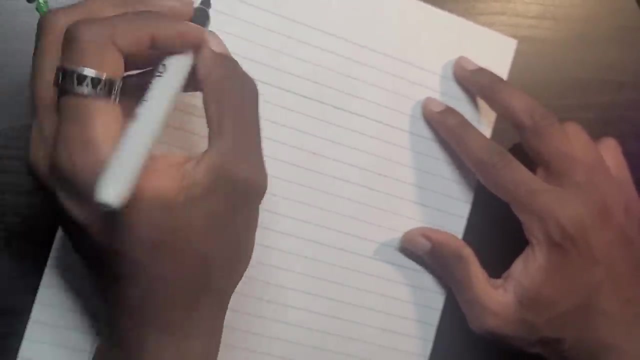 So let me just remove this paper right here And if you guys remember something you guys are again familiar with, let me start with something you guys are familiar with. If you guys remember when we were using the analog- I want you to focus here- analog right. 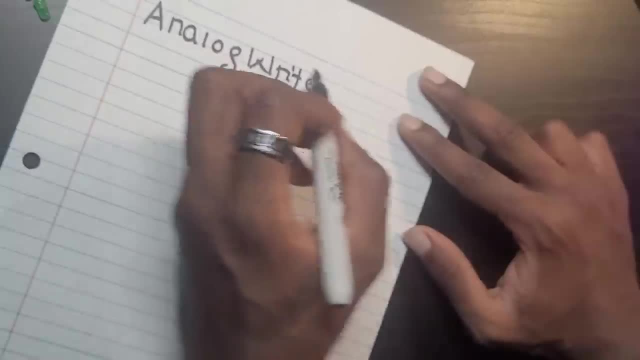 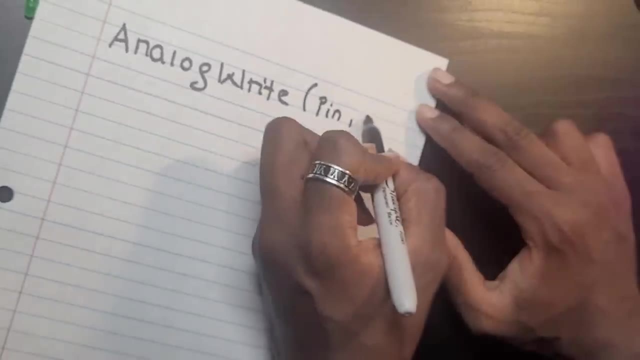 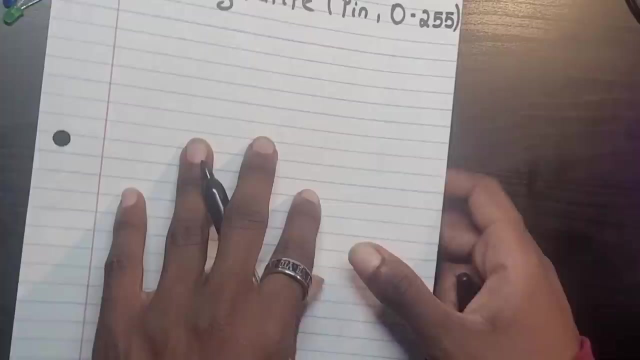 command. what did we do? We stated the pin right here- what pin were we using? and then we stated a value: from what? From zero to 255, if you remember- Wait, let me get the paper right here- From zero to what? 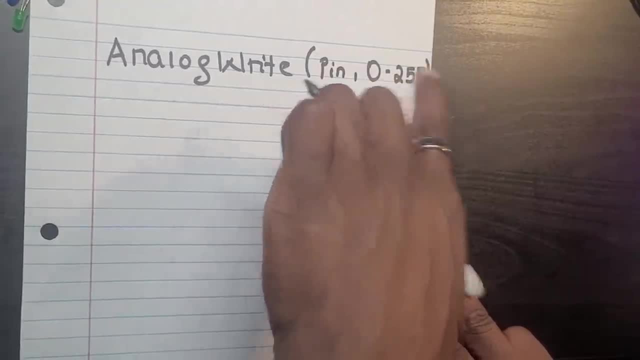 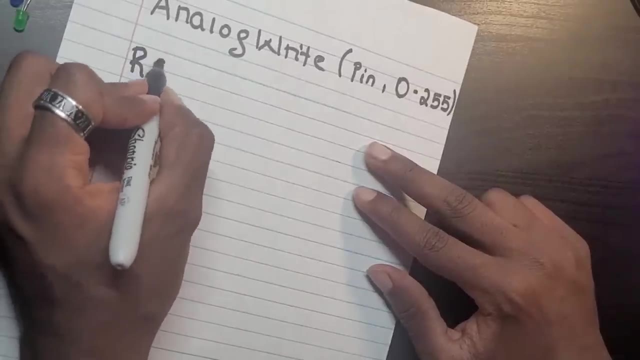 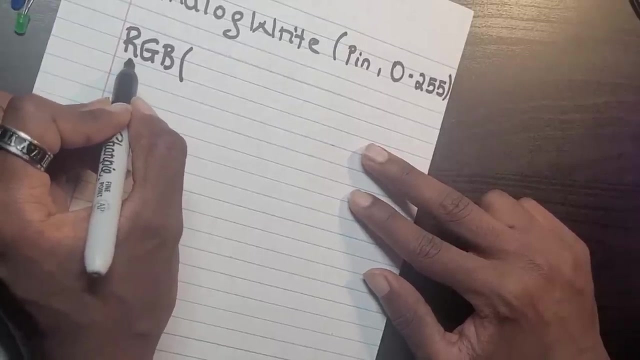 A number from zero to 255, an integer from zero to 255.. So one thing you need to know about RGB is literally what it basically means: okay When it's written in this form, it is okay. the first one represents red. 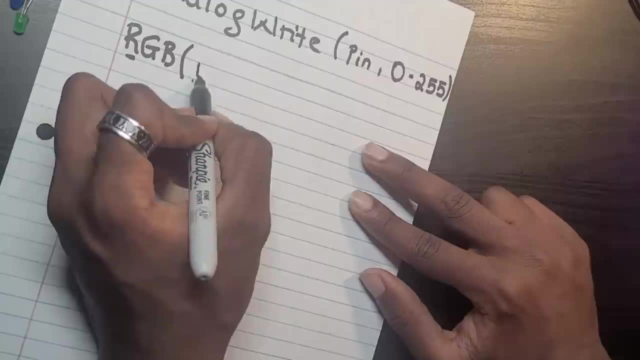 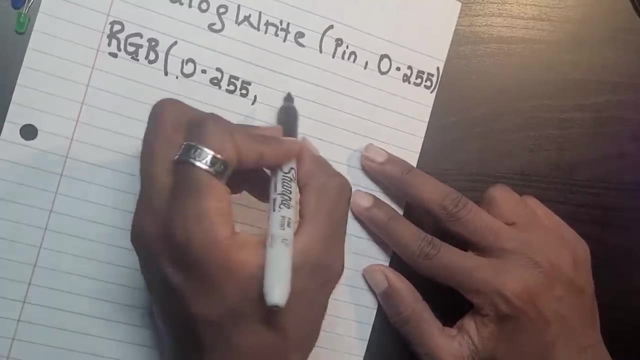 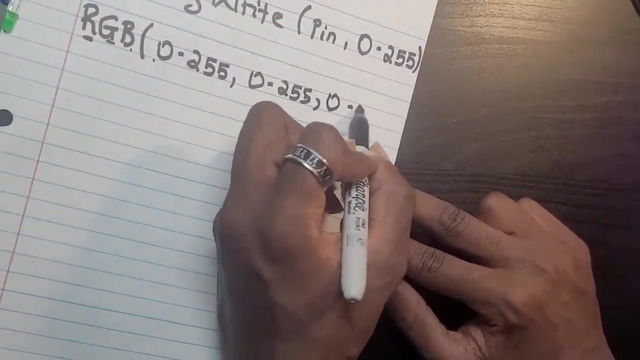 The first value represents the amount of red, And it's going to be from zero to what? To 255.. See that It's going to be the green one is also going to be zero to 255.. The third value is going to be a blue, which is going to be zero to 255.. 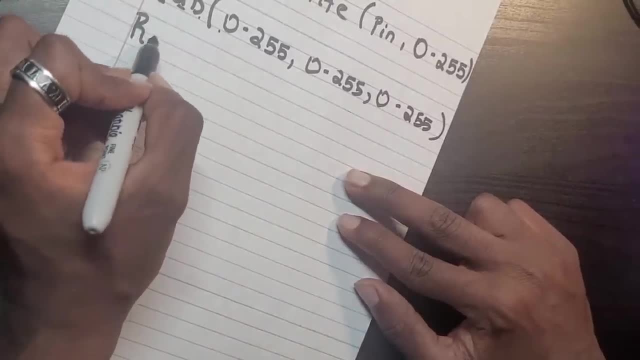 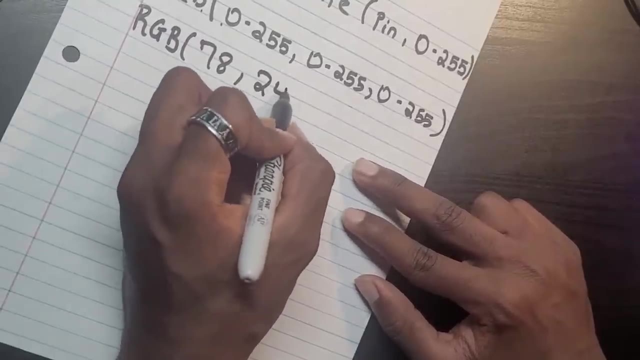 Okay, So if we have, let's say, a color, for example, that is written as RGB, let's say 78, 241,, 241.. Okay, Okay. So, let's see, this one is set to even zero, right here. 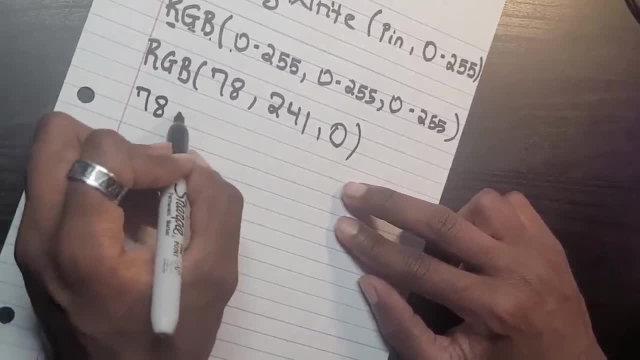 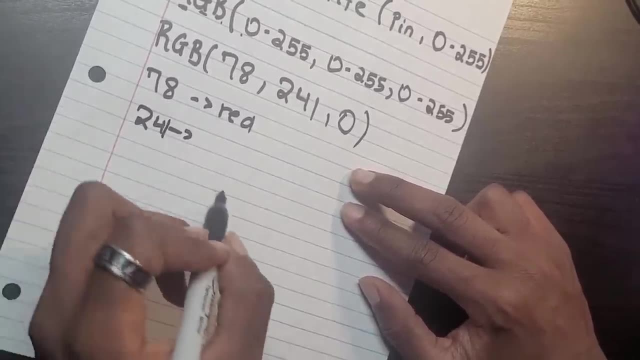 The 78 is what. The 78 is the value of what. The value of red. 24 is the value of what It's the value. So 241 is the value of what. It's the value of green: Okay. 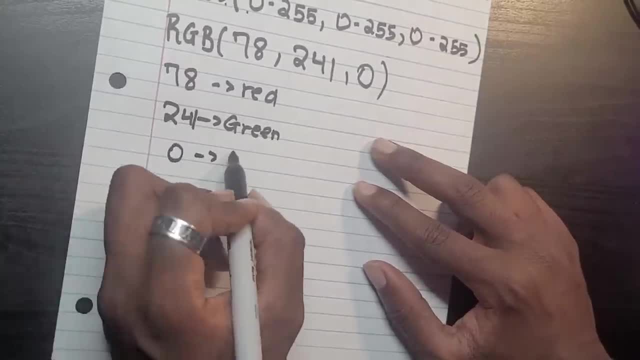 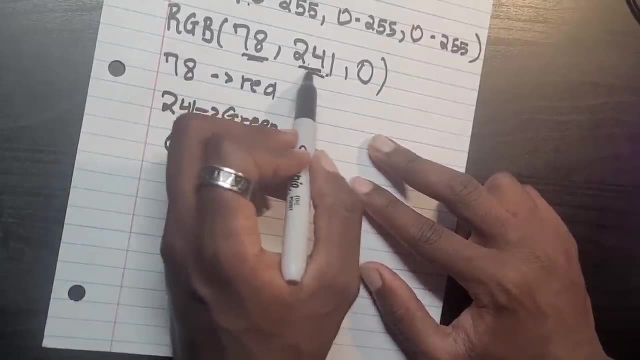 I want you to keep that in mind. And zero is the value of what? The value of blue. Okay, So the first value is going to be what The value of red, The green is going to be what The second value. 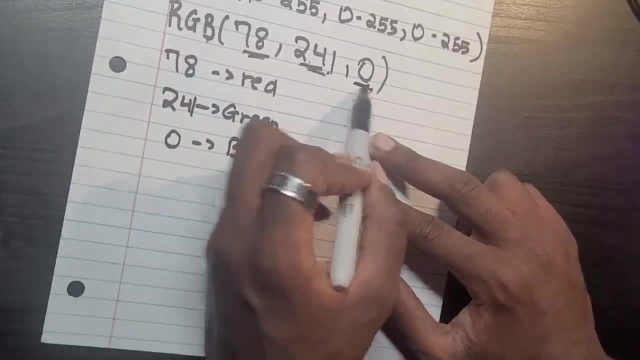 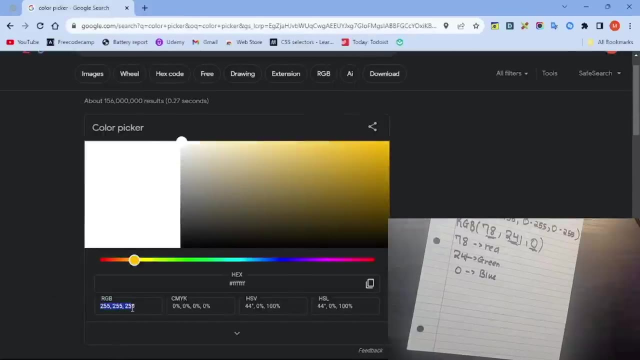 And zero is going to be what? Sorry, Blue is going to be what? The third value? Okay, We'll just keep that in mind. So let me go over to my screen right now. And when we see something as 255,, 255,, 255,, what does this mean? 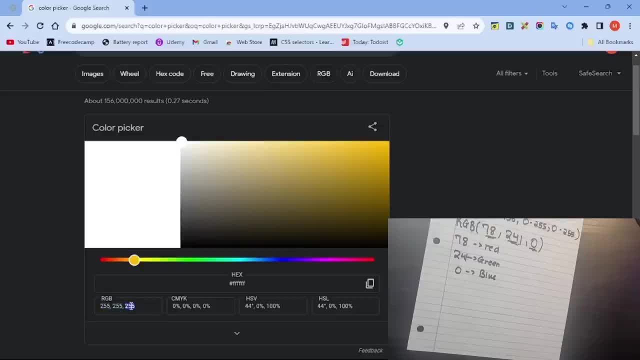 It basically means it's turned on to maximum. It's turned on to maximum. When we turn on everything to the maximum, what does it give us? The color white. So again, when we analyze the code- let's just analyze the code right here. 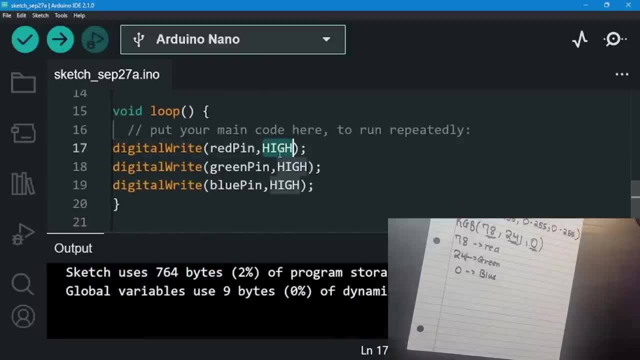 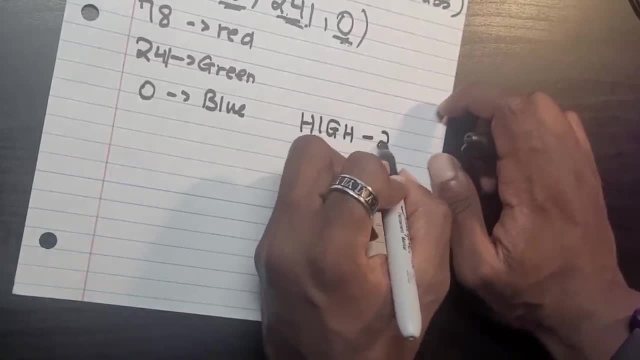 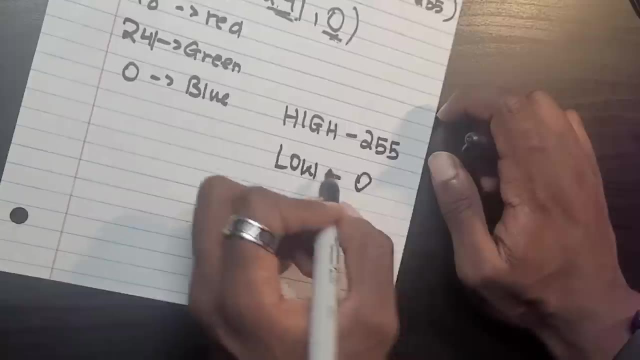 We just did. what Additional white high? What does additional white high mean? High means what. High corresponds with what. High corresponds with 255, as we learned again, What does low correspond with? Zero corresponds to what To zero? Basically, 255 means what? 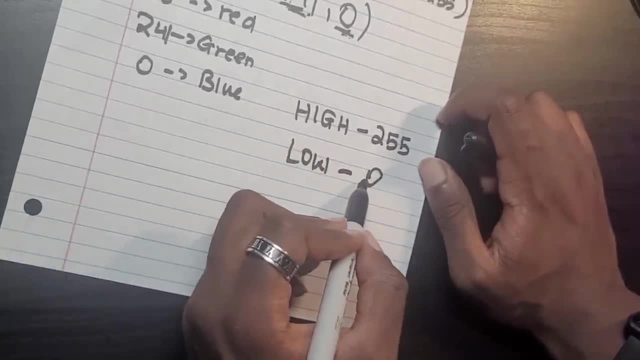 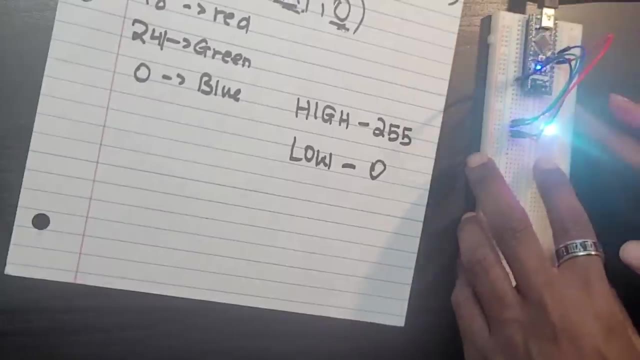 255 means 5 volt, while low corresponds to zero, which means zero volt. Okay, So we've just what Created? only white light right here. What we've created is what White light? But we can create many, many lights by using what? 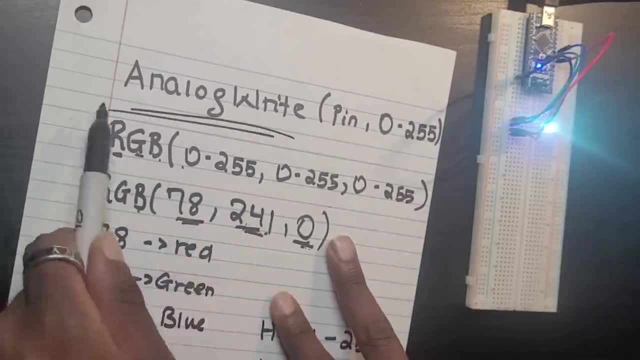 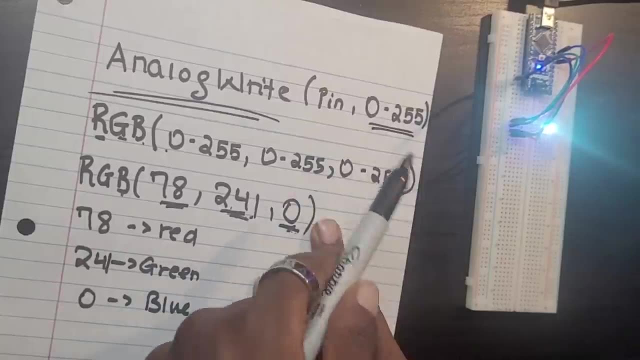 By using the analog write command, because what we can set it from a value to zero to 255. What we did is what Set? only zero to 255. That's all we could have done. We only can set it to zero or 255, but now we can set it to any number between zero and 255. 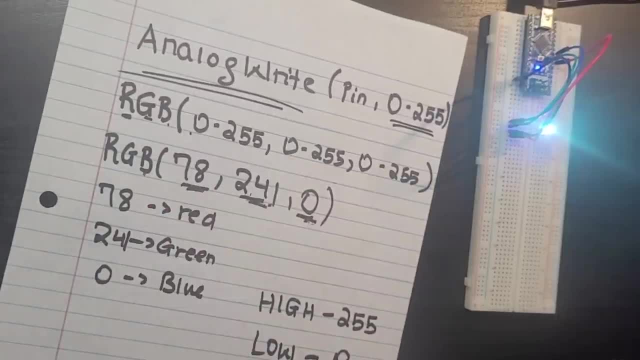 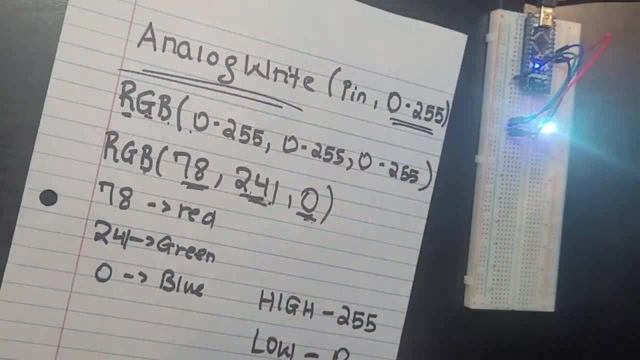 So when we use analog, right, we're going to be what we're going to be: unlocking new possibilities, Okay. So what we're going to do right now is we're going to first change the pins that we use, Again the digital pins. 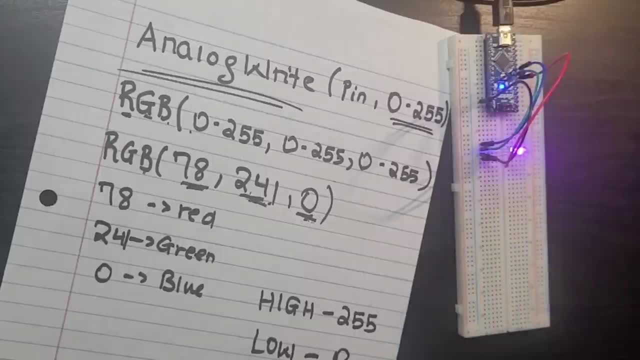 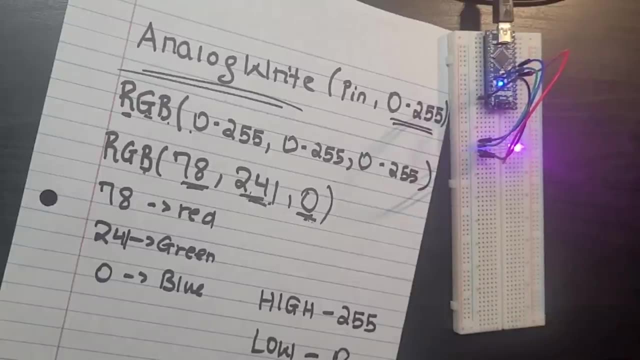 We're going to be Finding those squiggly line pins again that look like what. they're marked with the D and have a what a squiggly sign on them. I told you guys that this pins are what both- analog pins- and they both function as analog pins and as digital pets. 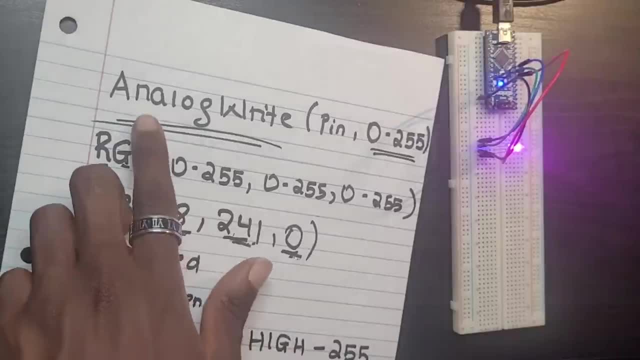 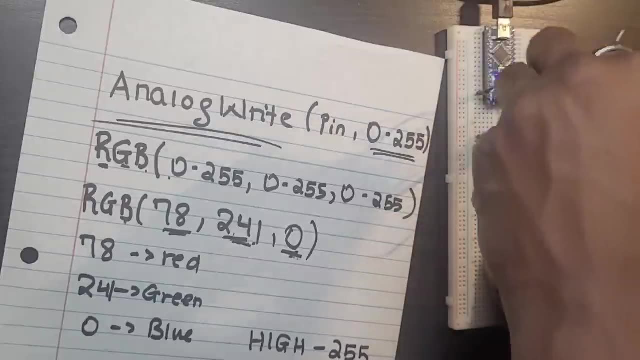 So let's try to find those squiggly signed pins and try to use analog right Command on them. Okay, So let's just do that. So let me just remove all of it, except for the G and D. the G and D always stays the same. 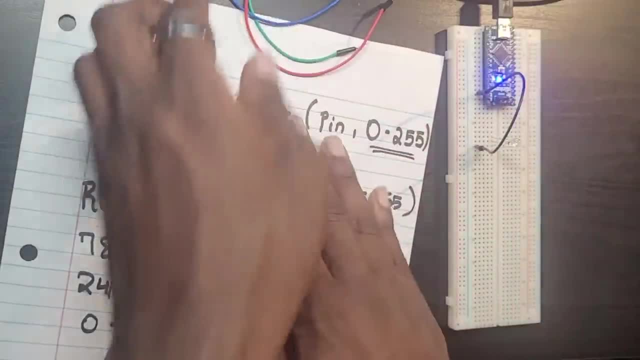 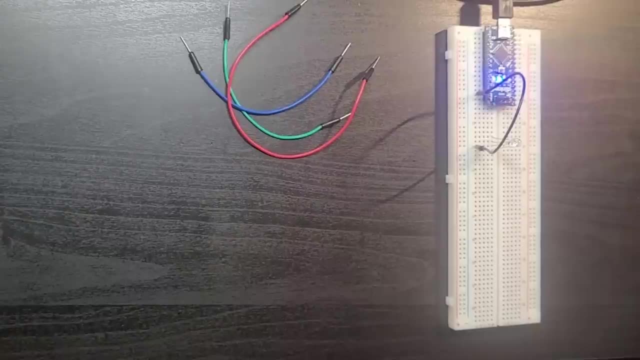 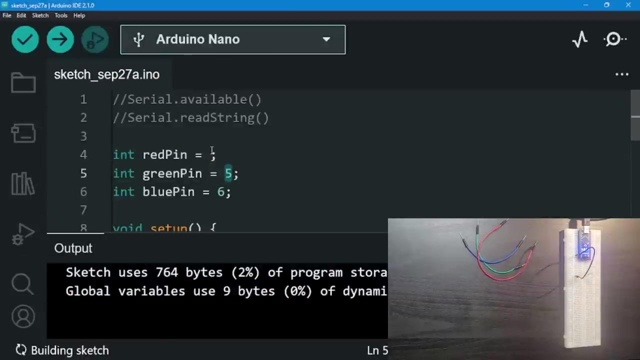 So I'm just going to keep it there. I'm just going to keep the wires here, because I'm going to get Back to them again. Let me just take off this paper for now, And what I'm going to do is go to my screen right here and we have to remove four versus move four, five, then six. 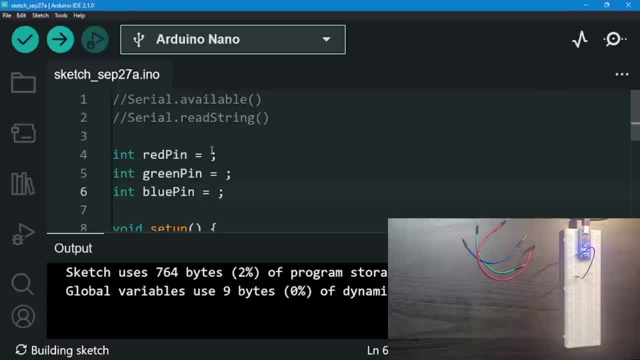 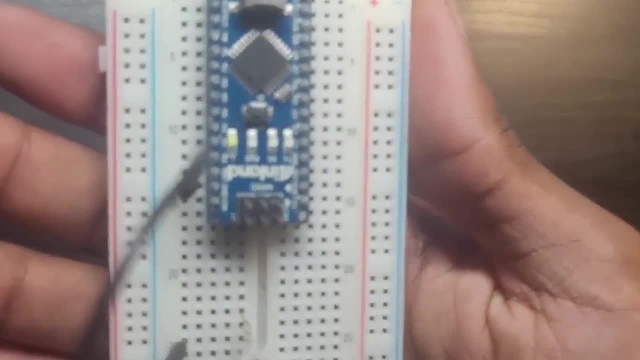 We're going to send them to what the digital pins that have? what the squiggly sign? So let's look at one that we have right here. So let me unplug my Arduino right here, because it makes no sense to plug it right now. 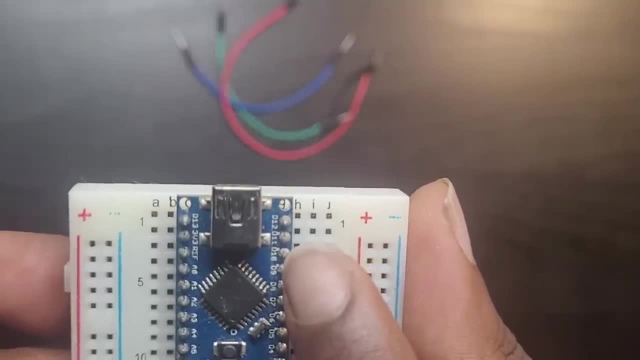 Okay, So let's try to find. mine is an Arduino nano, So we're going to look for what For a dot On the what On the digital pins. So let's look closer and you can see one on digital pin 11.. 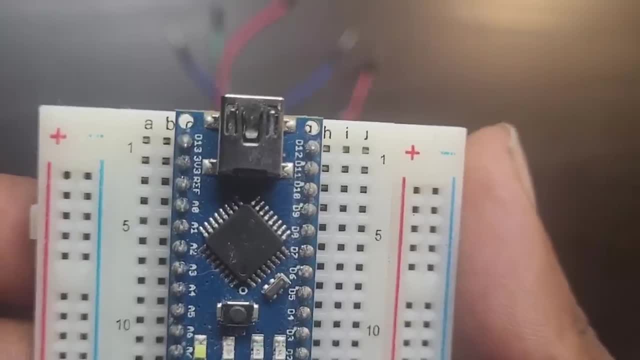 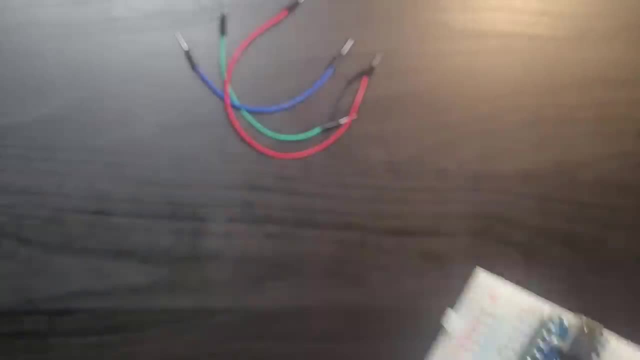 We can see one on digital pin 10 and we can see one on digital pin nine, So let's connect to these three, Okay, So there's still pin 10,. sorry, there's still pin 11,, 10, and nine are going to be the ones that I'm going to be using. 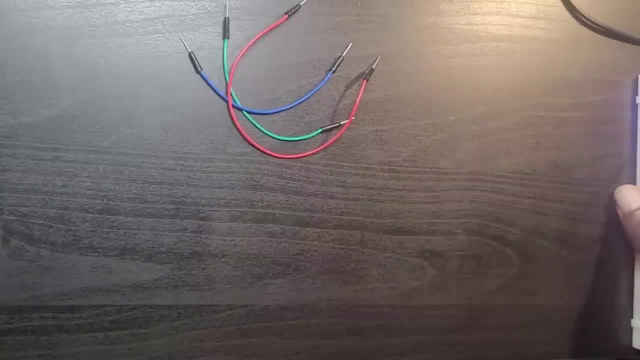 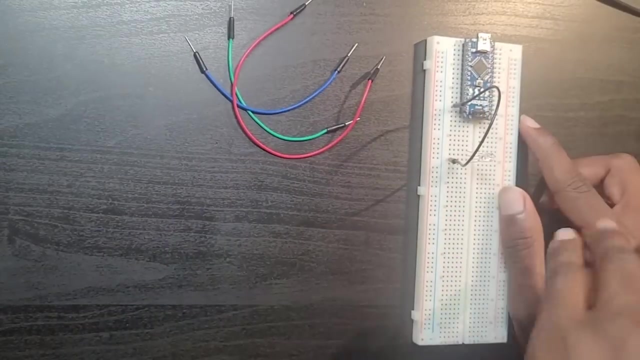 So let me just do that. Actually, I'm not supposed to be plugging my Arduino. I'm going to plug it and let's start working with. actually, let's first assemble it and then we can go and write the code. Okay, So, digital pin 10, I'm going to be setting it to digital pin 11.. 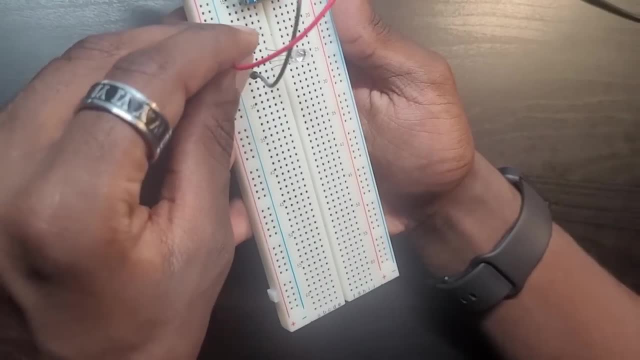 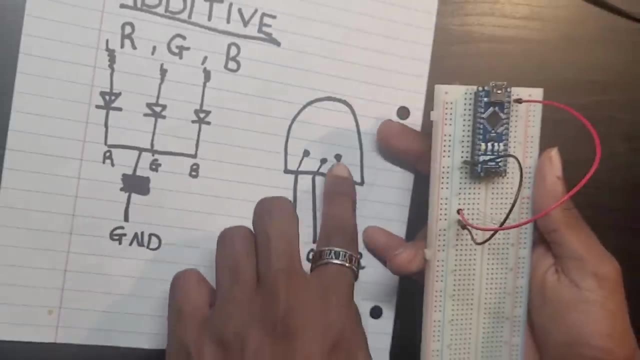 It's going to be set to red. I'm just going to do that. Let me just bring this here so you guys can again remember it: The red is what At the very very, what At the very last. So I'm going to be setting it to digital pin instead of digital pin 11.. 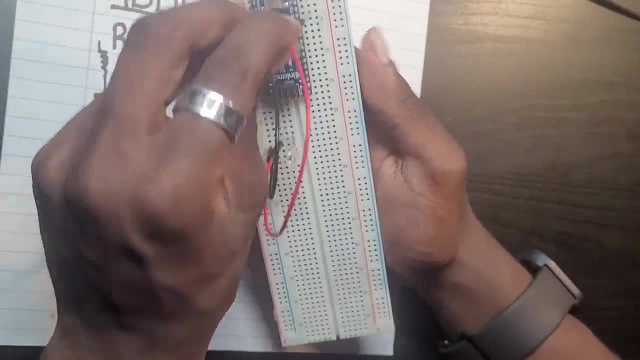 It's better to set it as digital pin nine because it's going to be closer. Okay, So I'm just going to set this to what? Digital pin nine. I'm going to change my mind and change it and change it to what. 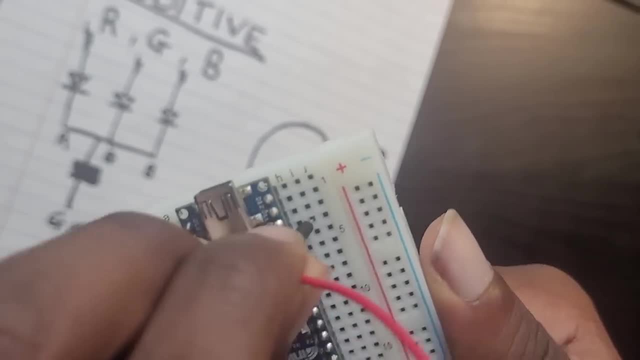 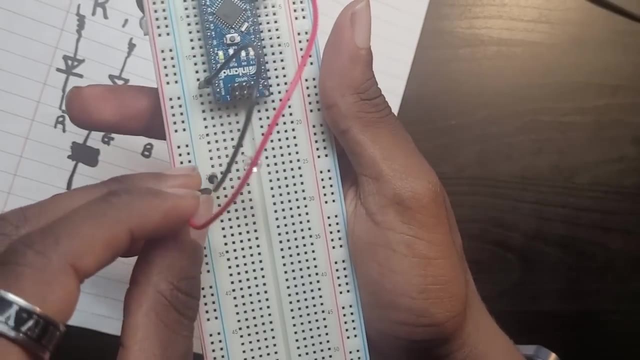 To digital pin nine. Let me just set it to digital pin nine right here. Set this to digital pin nine. Where am I supposed to connect it? Next to the GND pin, to the very right? So let me just do that. There we go. 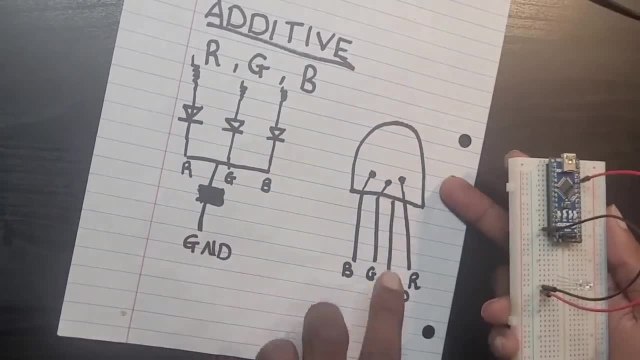 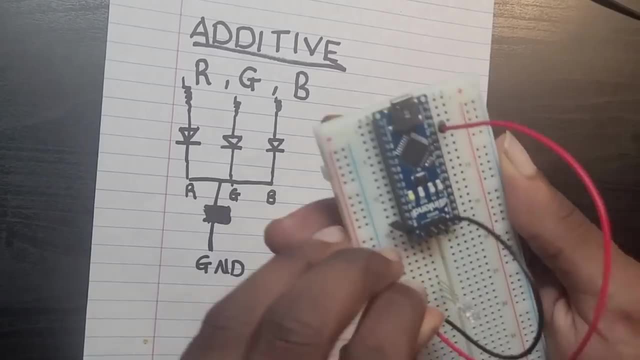 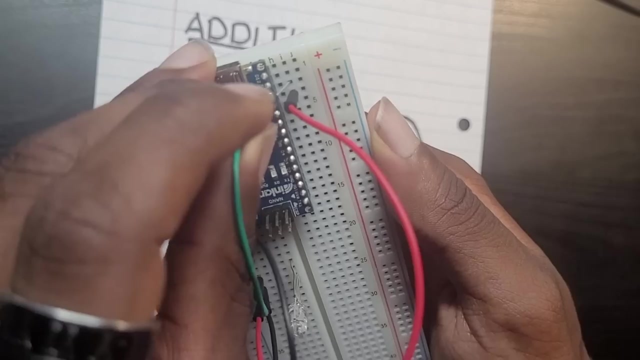 Connected it, Nice. Now what do I need to do? I need to set up green. Let me get my green wire right here. Let's find my green wire and put it right here. I need to go to digital Pin 10.. 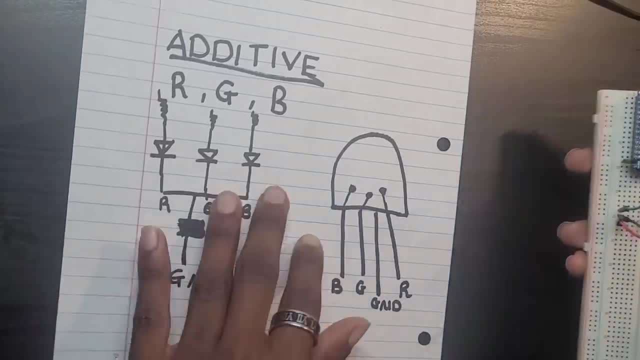 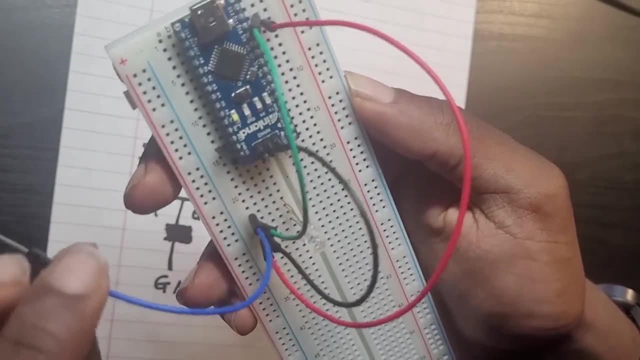 I'm going to go for digital pin: 10 for green. Okay, Then I'm going to go for the blue one, which is going to be the most left one. There we go, And I'm going to set it up for what? 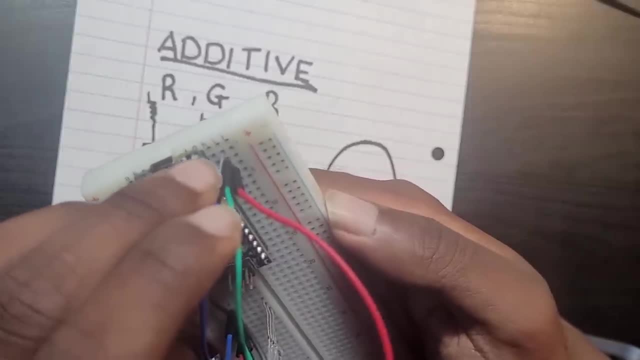 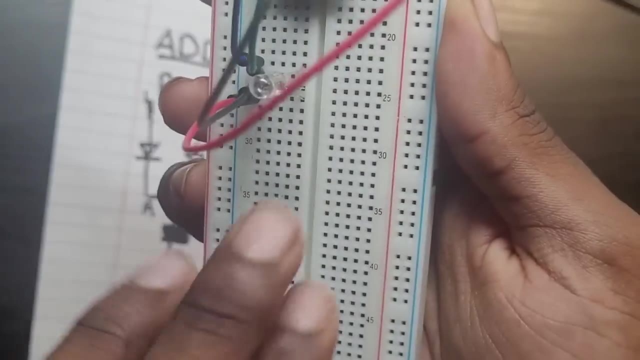 Digital pin 11.. Oh, the space is very tight. Let me just do that. There we go. You guys can see it right now. Let me just do that, Let me just make sure that you guys can actually see everything, every setup. 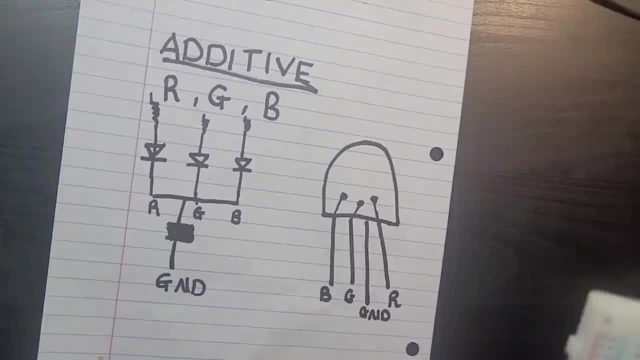 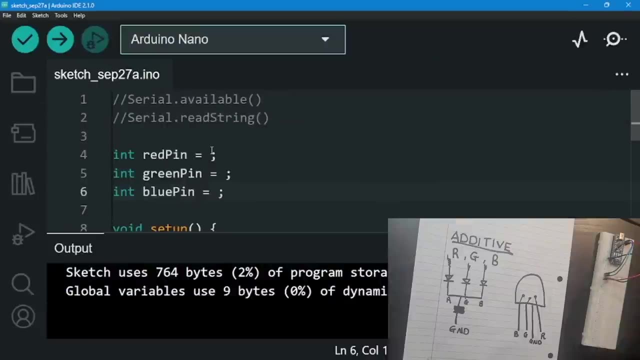 And there you have it. Okay, So now what I'm going to do is: let's go over to my screen and let's start writing the code. Okay, So the red pin is set to what? Digital pin 9.. While the green pin is set to digital pin 10,, if I'm correct. 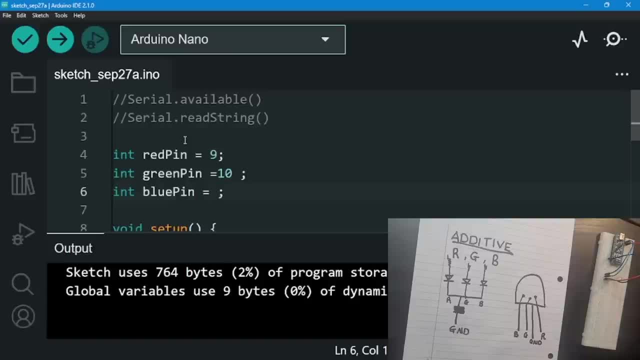 Digital pin 10.. There we go, And blue pin is set to digital pin 11.. There we go. Now, what do I need to do right here? I'm going to be using them as an output, So this is all correct. 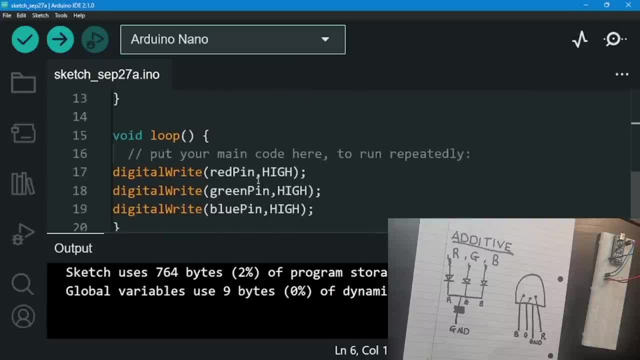 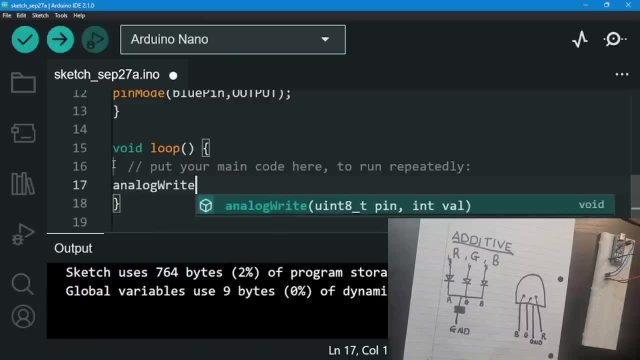 I'm not going to change anything here. What else am I going to change here? I'm going to be using what Analog write instead of digital write. So I'm just going to do that Down- analog write- And I'm going to set to what. 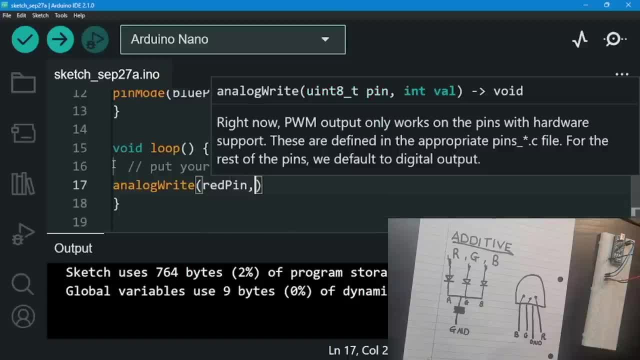 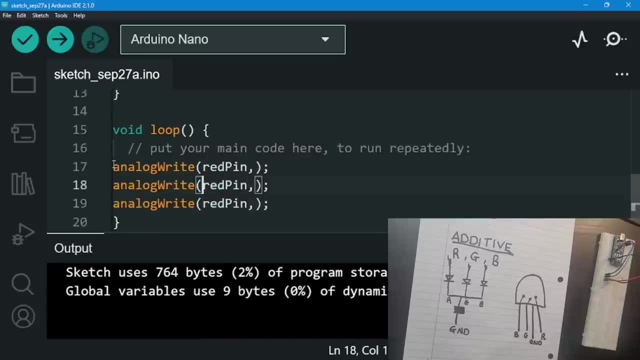 The first one. Let me just set the red pin to what? To some sort of value. I'm not going to do that right now. Well, I'm going to set it up. So let me again copy this: Set up green pin. 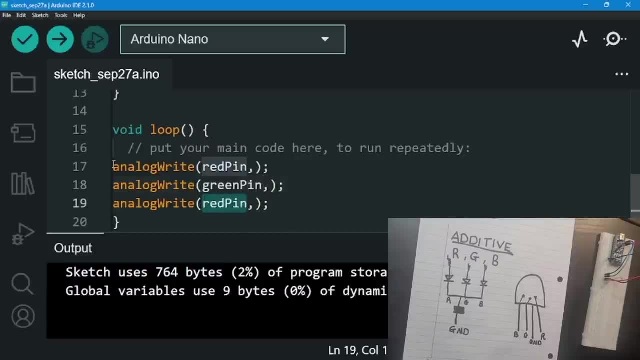 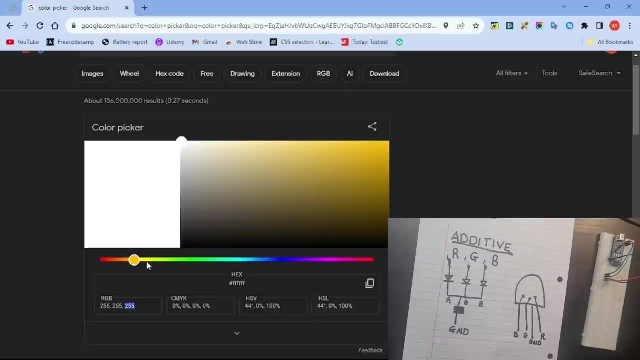 I'm going to set a value later And we have the blue pin. Okay, There we go. So now, what I'm going to do is I'm going to go to my color picker right here. Okay, So, as you can see, we have the value right here written down on RGB. 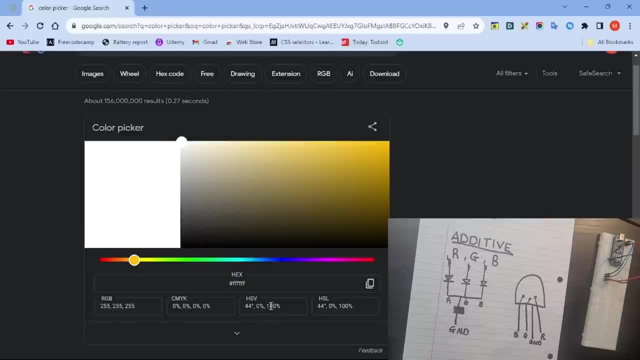 You can also see other values, such as CMYK, HSV, HSL. We're not going to get into them because we're not going to need them right now, But we're going to focus on RGB because this is going to be one of the most popular type of what. 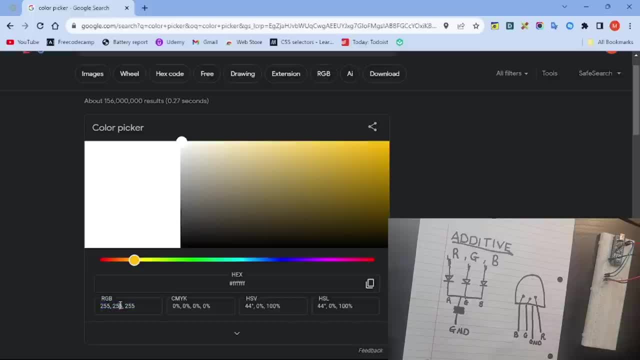 Color naming systems: All right. Not a color. what A color system. All right. So I just want to go for something more. I'm going to go for yellowish today and just be like something yellowish. Let me just go for something yellow. 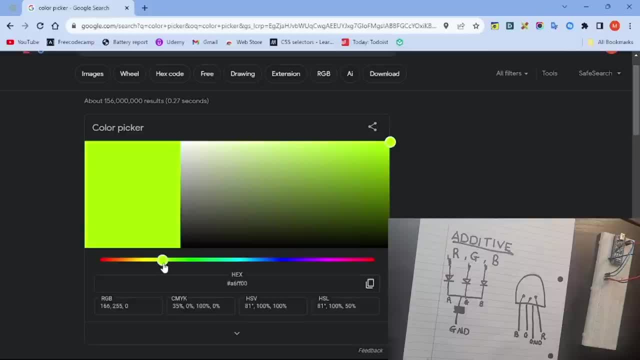 Okay, There we go. I like this color. I want it to be a bit brighter, though. Just make it a bit brighter. Actually, that looks good. I want it to be somewhat greenish, though Let me just go to the greener side of it. 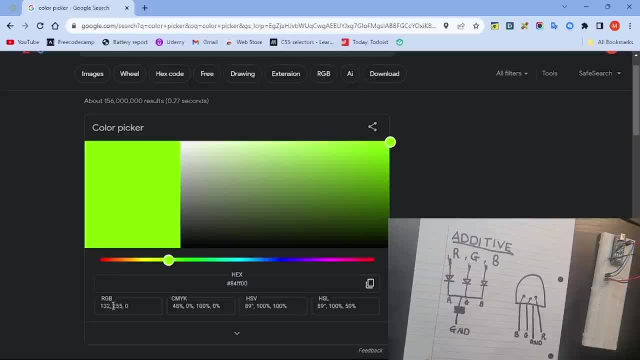 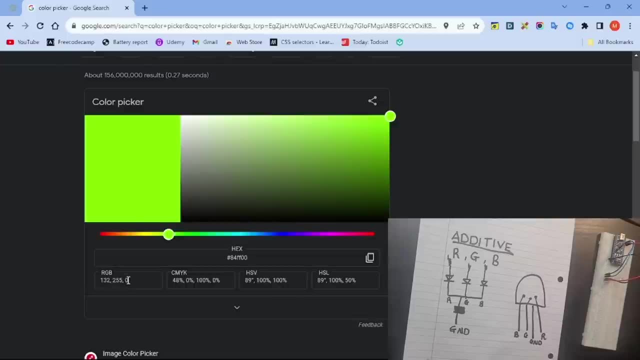 Okay, That looks nice. I like it. So what I need to do right here is, again, the RGB says that I'm supposed to set it what? 132 for red, 255 for green And zero for what? For blue? 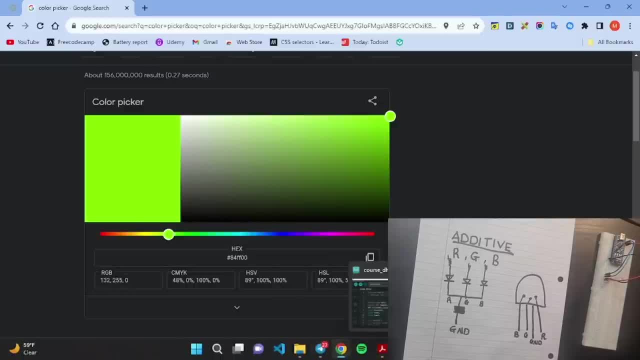 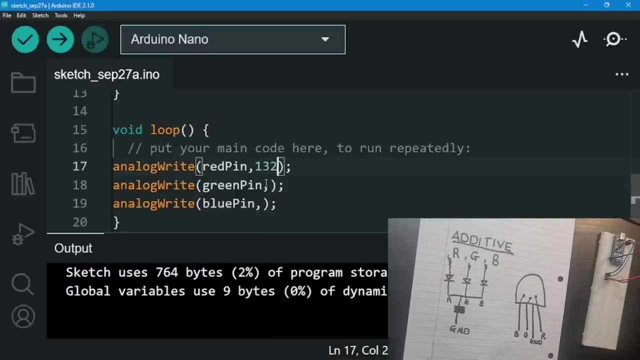 So let me just do that. Let me go over to my Arduino IDE. It's supposed to be right. here I have to set 132 for the red pin, 132.. For the green pin, I'm going to set it to what? 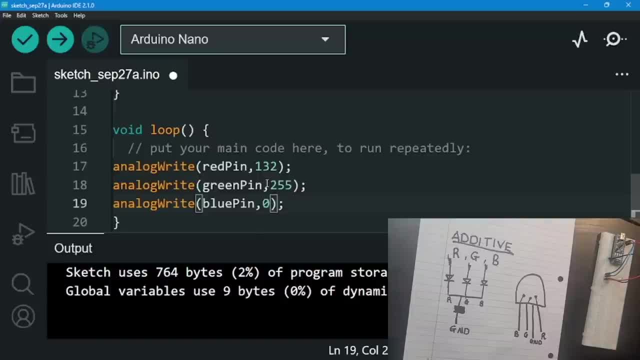 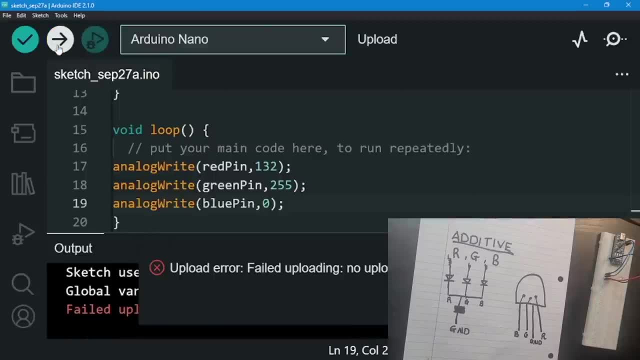 255.. And for the blue pin, I can just set it to zero. Okay, So all I need to do is upload this. Everything should be working. No upload port is provided. Why is that so I did not plug in my Arduino. 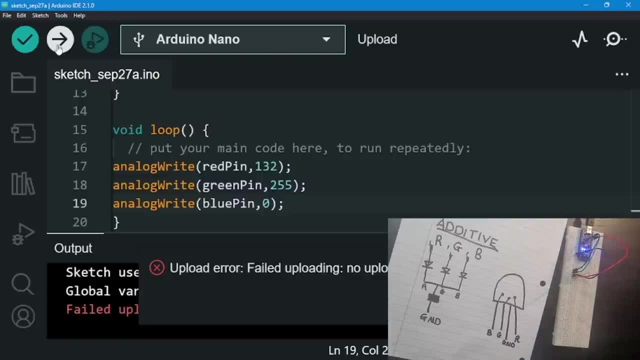 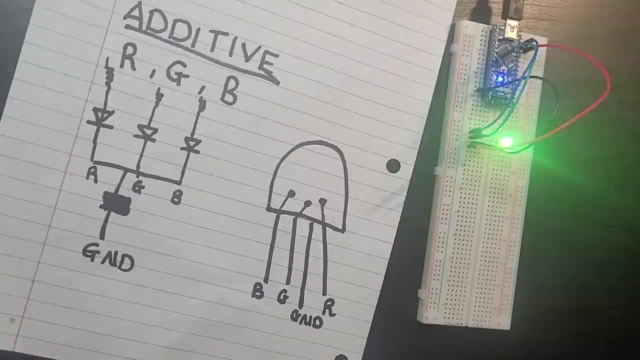 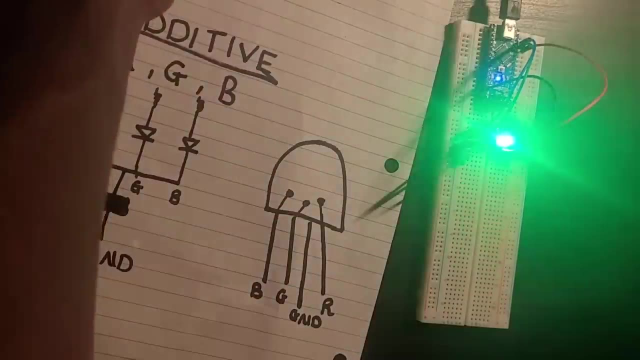 Let me just do that. Forgot to plug my Arduino right here. All right, Now let me try to upload it. Okay, It's done uploading, So let me just turn off the lights so you guys can see it way better. Again, turn off the lights. 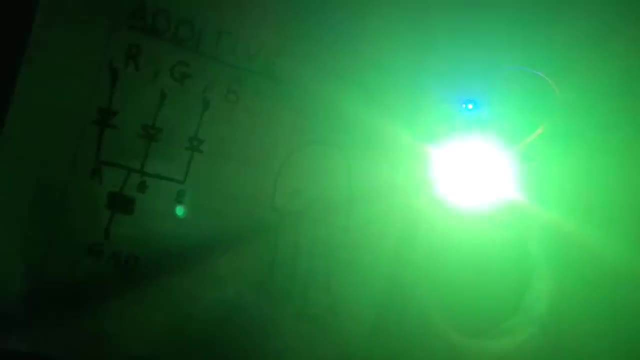 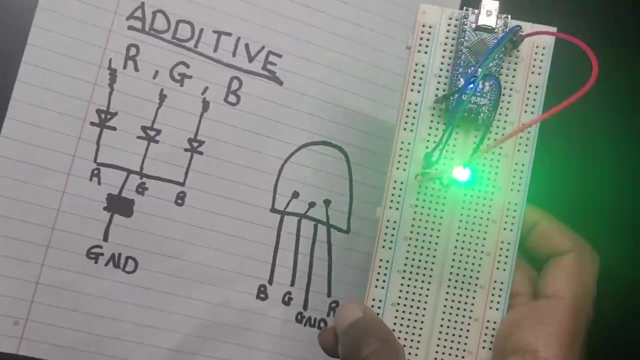 It's really hard actually when there's a thing, Turn on the light. actually It's way better with the light. At least it's not going to be too bright that you cannot see it. It gives me the yellowish. 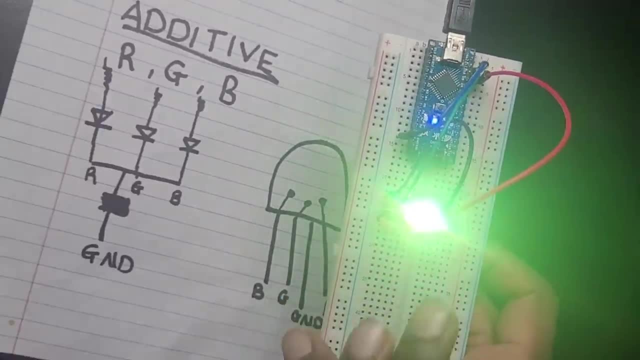 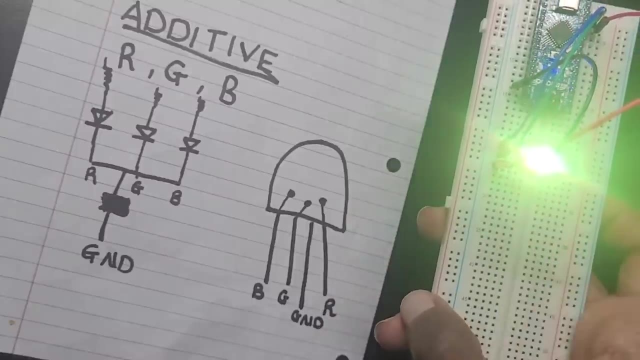 You cannot see it again because of the screen. again It's going to focus on only one light, But if you look at it it looks like somewhat yellowish type of green. It doesn't look like the one that looks on the screen like perfectly, but it looks somewhat. 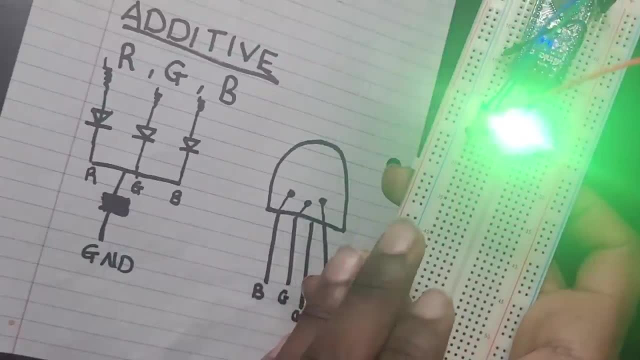 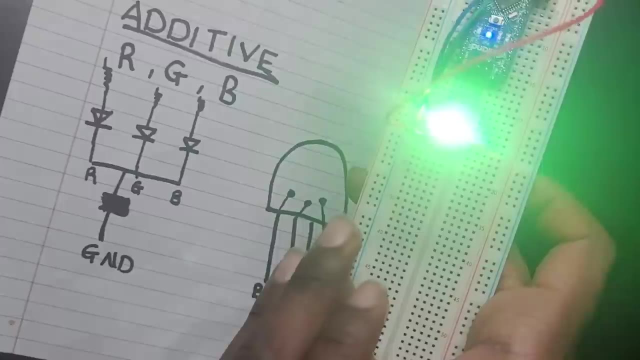 yellowish type of? what Type of green right here, Some yellowish type of green. If I rotate it to another degree it looks like yellow. You can see that right. If I rotate it to a degree it looks like a yellow. 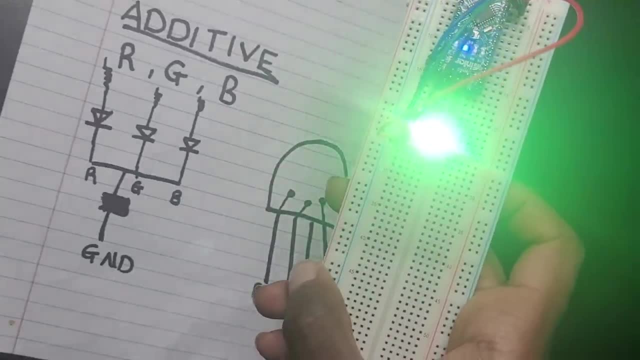 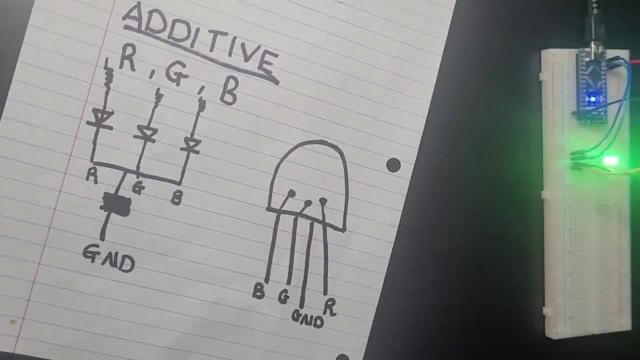 When I rotate back to another degree, it looks like green. There we go. It looks like a green right here. Okay, So right here, let me just try to make something of a distinct color. Let me just again turn on the light. 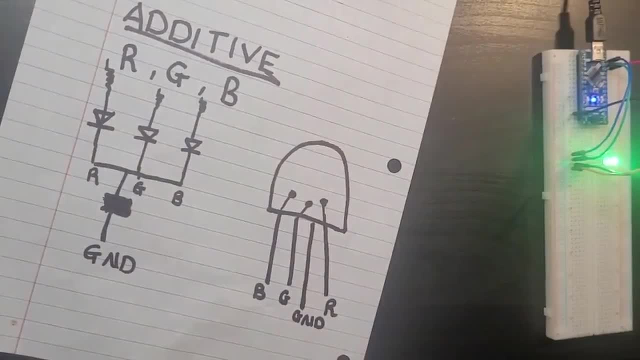 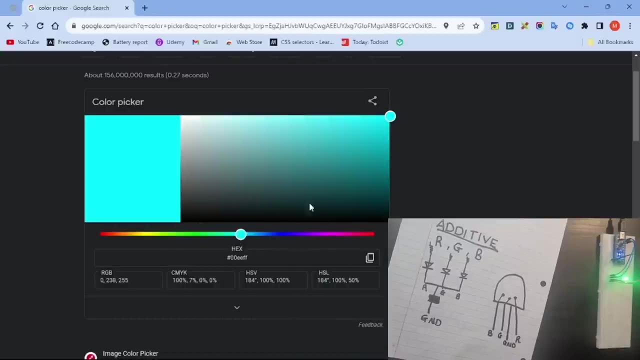 Let me try to make somewhat of a very distinct color that we don't have. We already have a yellow pen, so let's try to find something that we don't have, maybe a color that we don't have, Maybe something like cyan, because we don't have a cyan type of color right here. 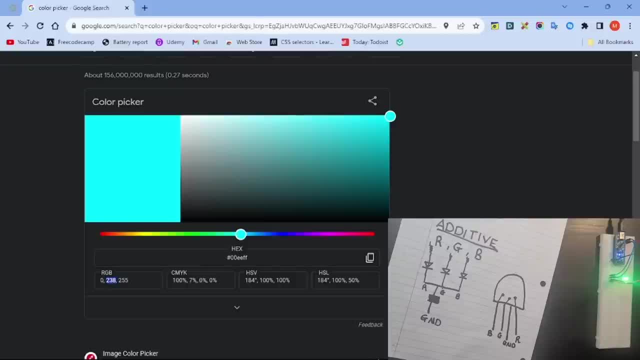 Cyan is one of my favorite colors. I actually like it so much. Okay, So the value of cyan is what? Almost what? 238, 255.. But if you go to the closer side, actually it's going to be 255, right here. 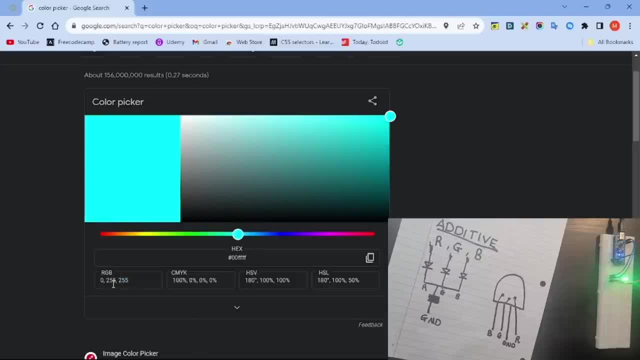 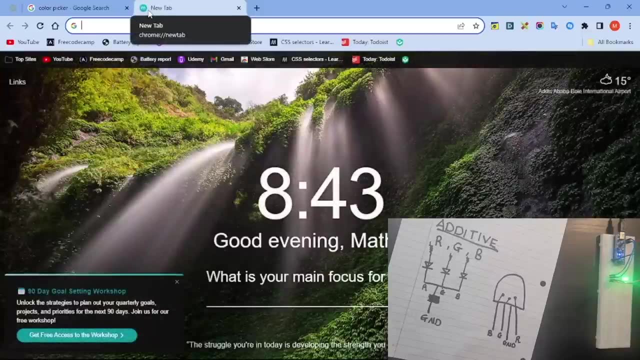 The most cyan color is going to be 255.. There we go: 255.. This is cyan. If you want to find, for example, by the way, if you want to find a specific color, okay, if you want to find any specific color, the RGB value of any specific color, all you have. 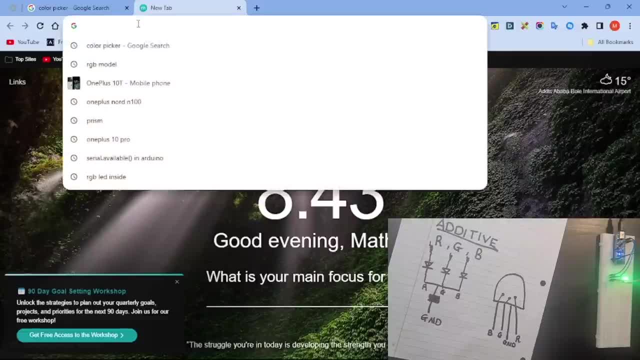 to do is what All you have to do is Google it. So, right here, you're going to go right here and say: Let's say I want the color pink. Okay, So I'm going to say it's pink. 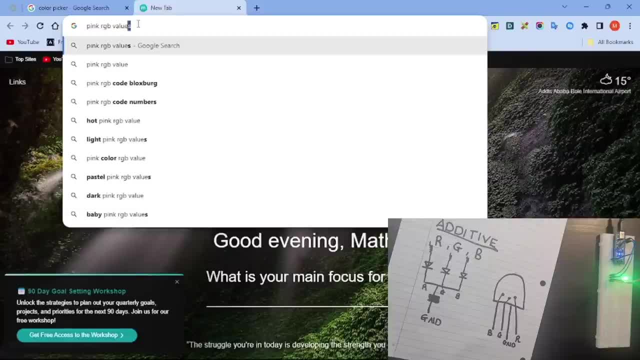 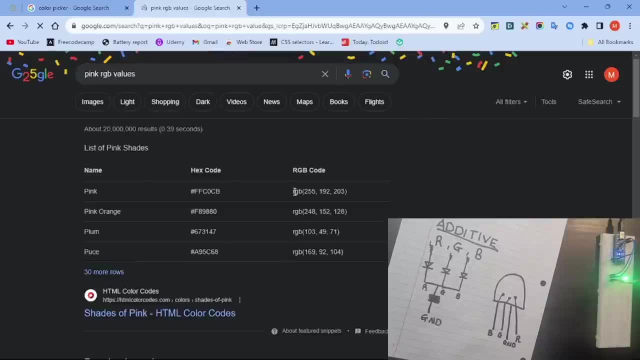 What I'm going to say is pink RGB value or RGB code. It's RGB code or value. We need to just do that. The pink is going to be right here. The RGB code is what? 255,, 192, and 203. 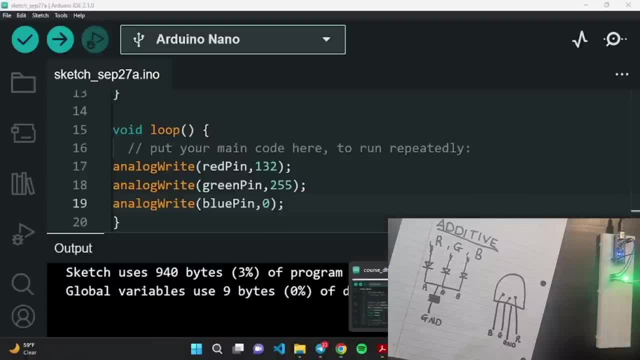 All you need to do is go right here. Okay, So I'm going to set the red to 255.. Let me just do that: Set it to 255.. And this one to 192.. All I need to do is set it up to 192, if I'm correct. 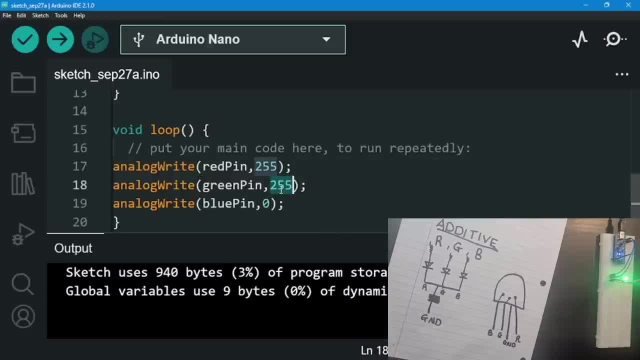 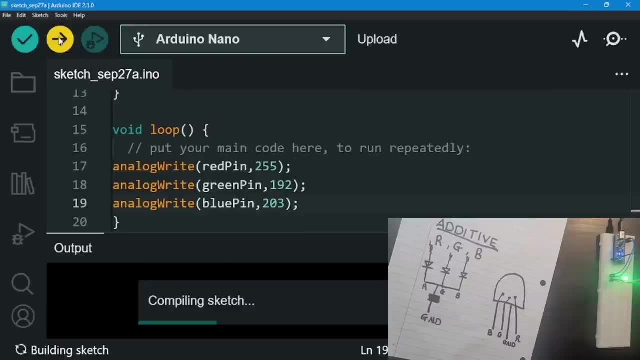 Let me just look over 192,, 192, and this one to 203.. There we go. All I need to do is what? Upload it right now. Let me just do that. It's done compiling And now it's uploading. 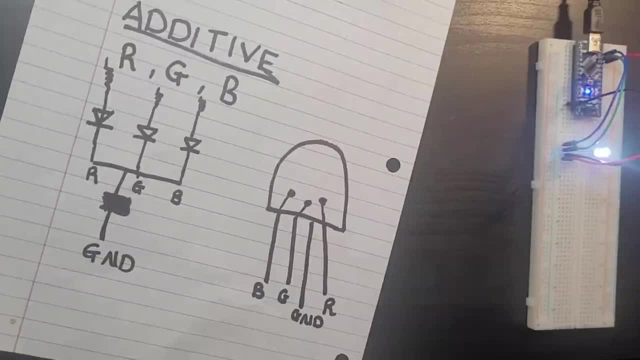 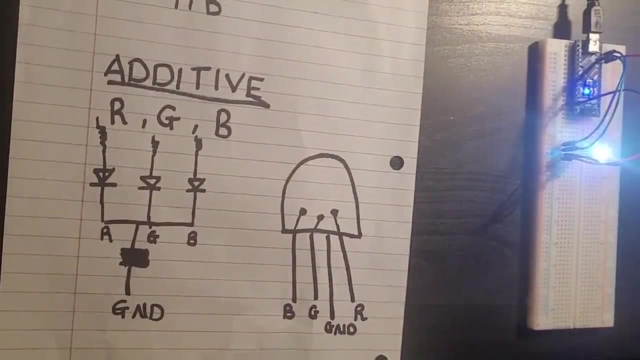 It's done uploading, As you can see right here. let me just turn off the lights, if it helps you. It looks somewhat like white right now. Let me just turn off the light so that it can help. Let me just do that. 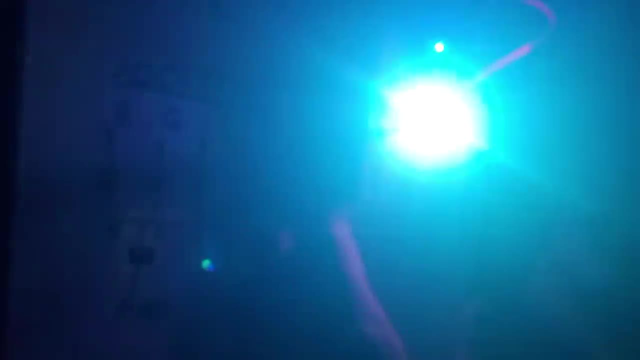 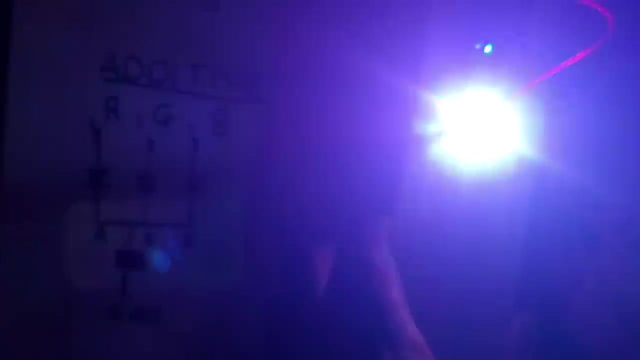 Okay, So again, it was really a hustle. You can see that the color is changing a lot. It's changing from green to, right now, red when I tilt it again, and now to a blue. But if I go in the right direction right here, it doesn't look like pink right here. 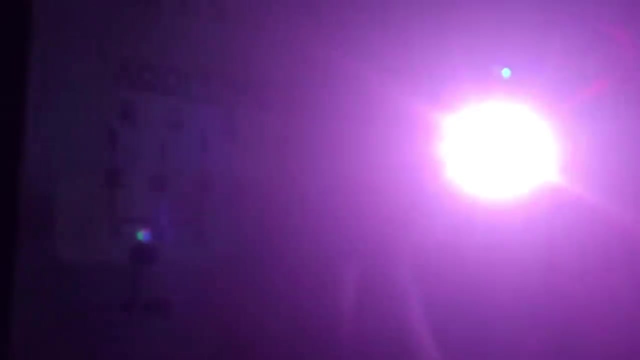 It looks like a pink right here. Can you see it? A pinkish color? I can see it right here. It looks somewhat like pinkish. by the way, You cannot see it that much because, again, we're using camera. 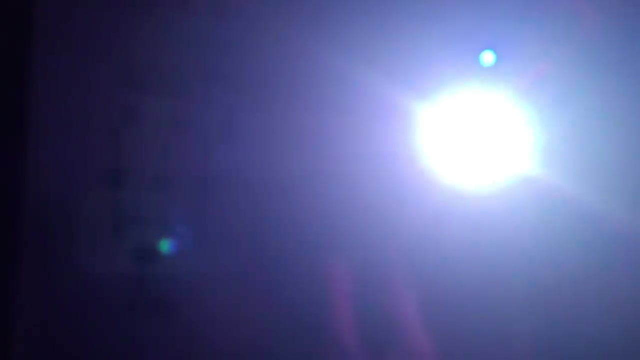 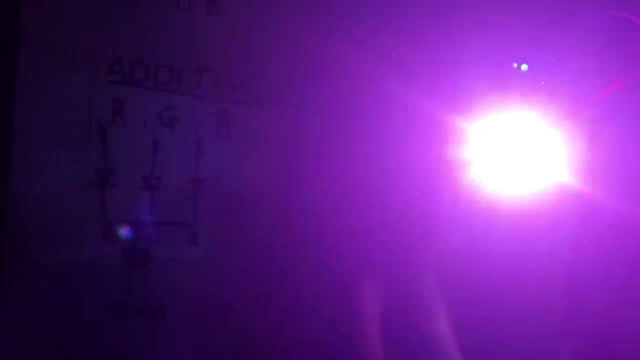 But you can see what Somewhat of a pink when I tilt it. When I tilt it to the right degree, you can see somewhat of a pink. There we go Somewhat of a pink right here. There we go, We got pink. 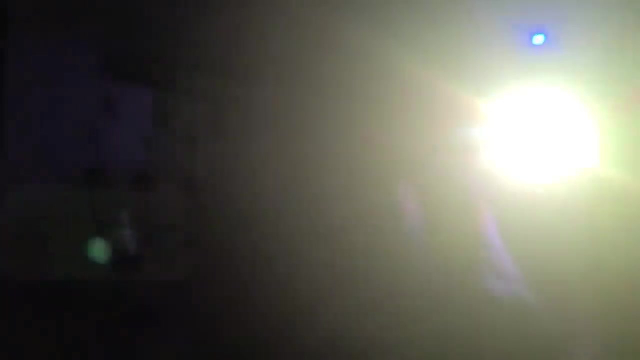 That is beautiful. Let's just do that. Can you see it? It's beautiful, All right. So again, you guys can choose any color you want. Google it Again. any color you know, maybe indigo, cyan, any color you like. 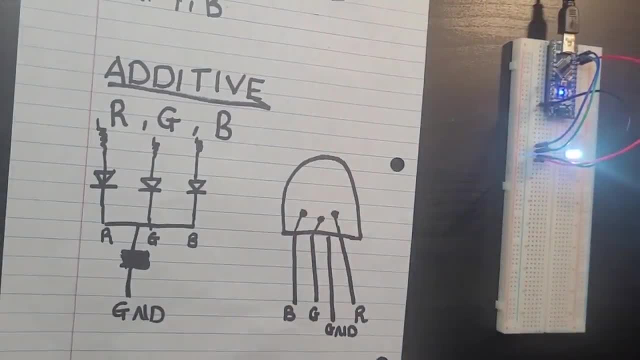 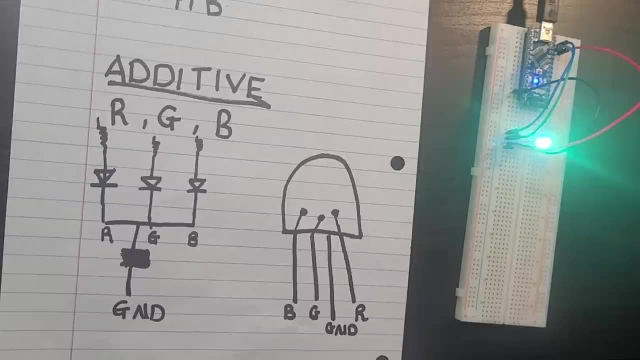 Google it, obviously, And yeah, all you have to do is search for this. You can search for the RGB value and you can again do what You can use your RGB LED and what, And try to create that light for yourself. 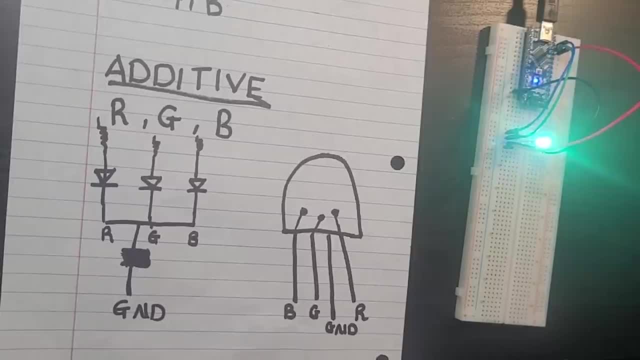 All right, I think this is it for this section of the course, But we're going to be working with RGB LEDs and adding up. We're going to take them to the next level by working with a serial monitor on the next section of the project. 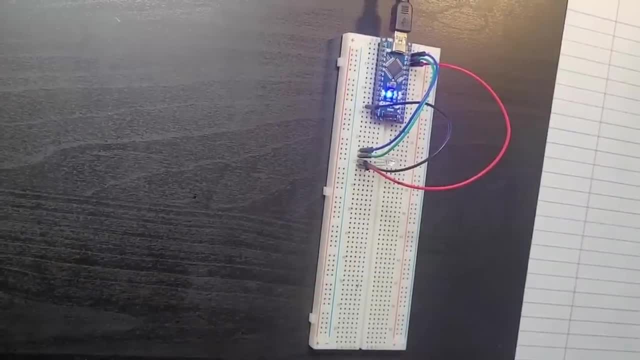 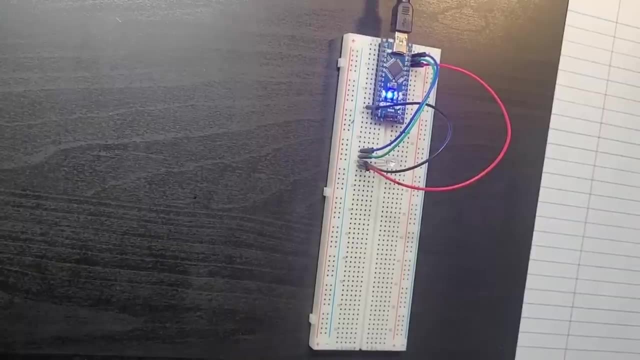 So see you then. Okay, So let's stop this part here. This project, as I said, again up a notch. So everything here is going to be the same. The components here are going to be the same. 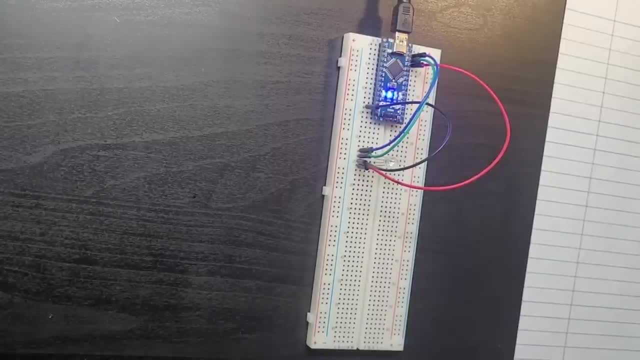 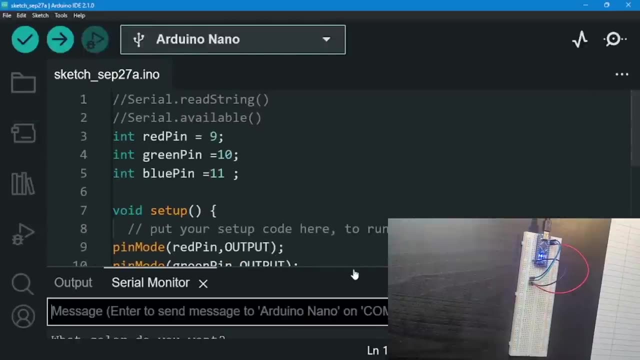 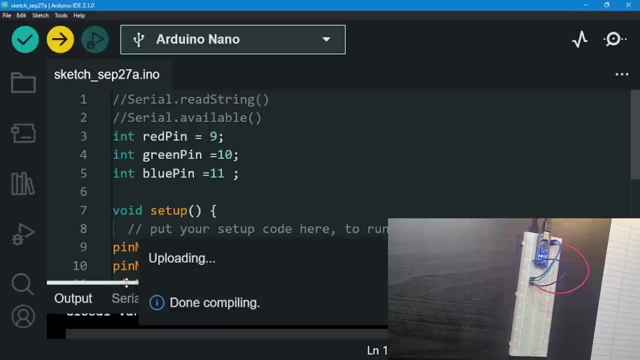 So is going to be the code. So we're going to continue what Where we left off, Okay. So right here, what I want to do on this project is use our serial monitor right here, Okay. And what do I want to do is let me actually upload this code right here. first, because I was working on the pseudocode. 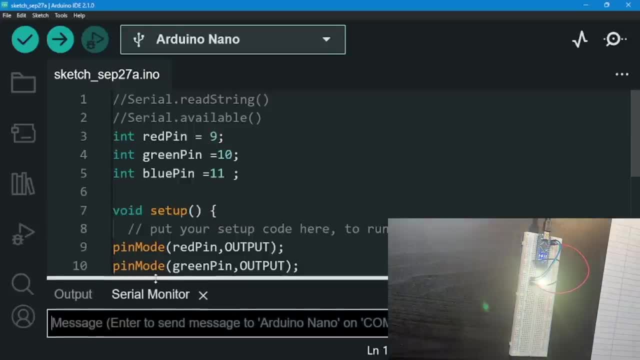 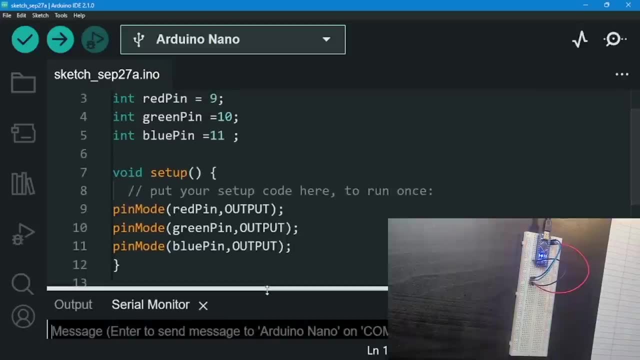 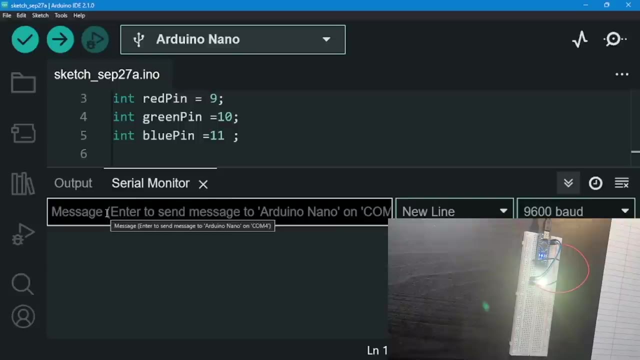 I was working on the code previously. I don't want to interfere with this one. Okay, Serial monitor should be printed now. Serial monitor should be like new. All right, There we go. And what do I want to do right here is okay. what do I want to do right here is I want to enter a message to what? 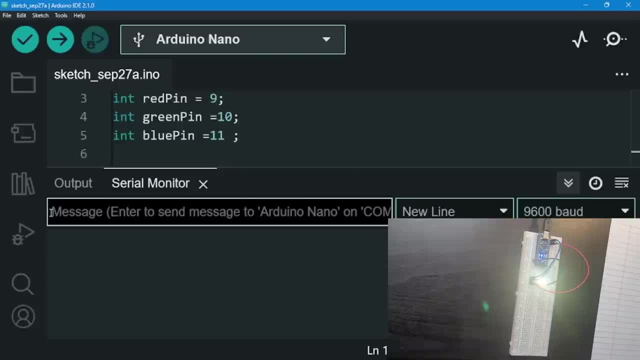 Our serial monitor, Okay, So, as you can see, right here there's a black bar that says message enter to send message to Arduino Nano. So, basically, we can use our serial monitor Not only to read, not to only what. 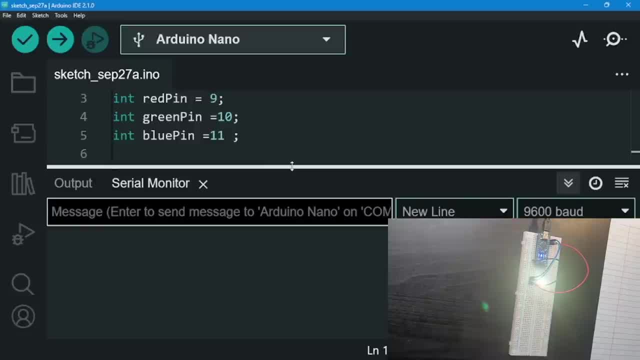 Listen or read from Arduino Nano, but we can use it to write messages. to what? To send messages to our Arduino Nano, basically to our Arduino. Okay, So how do we do that? Let's write down a message right here. Let's say: I said, read right here. 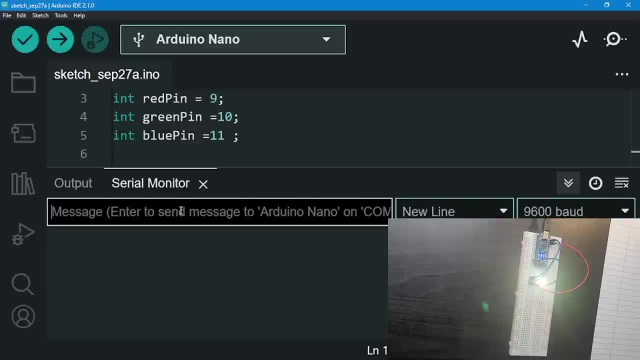 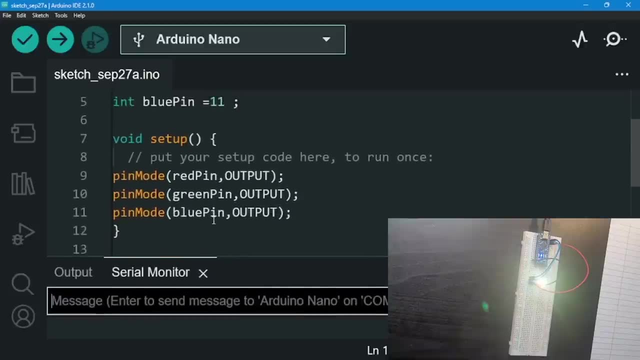 I can send it to what? To the Arduino. Obviously, right now it makes no sense because obviously we have to what We have: to create a system on which how we're going to receive the message and what Arduino should do when it receives the message. 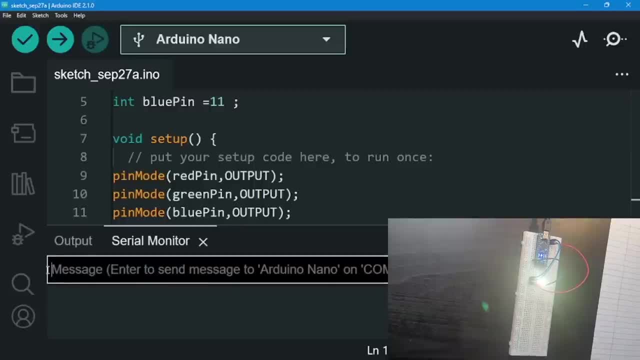 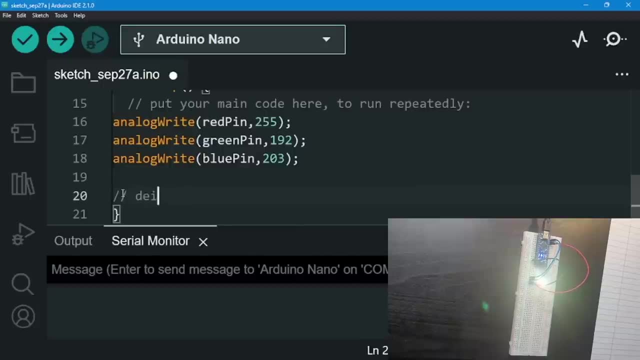 Okay, We don't have to set that code up. Anyways, we can set what messages, though, Just like how we have. I want you to think of this, just like how we have digital write it down properly: digital write and digital read. 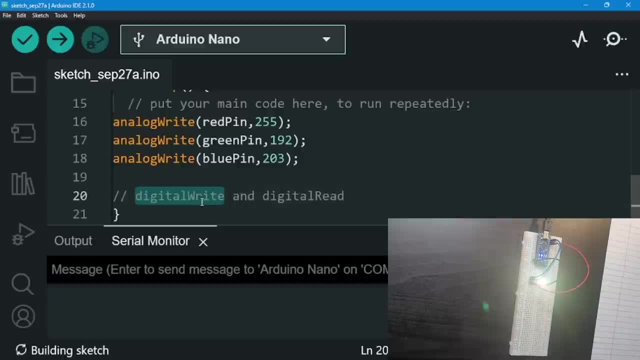 It's like how we have that when we can write the message to again using our digital pin and we can read message using our digital pin too. The same goes for analog too. We had what Analog write and analog Read. Now we're going to have is what. 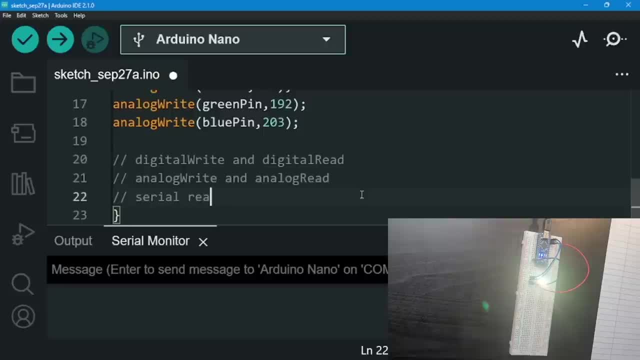 Now we're going to have a serial what We've been using what Serial read, We're reading what Using our, what, Our serial monitor, And now we're going to be using what Serial kind of something like what. 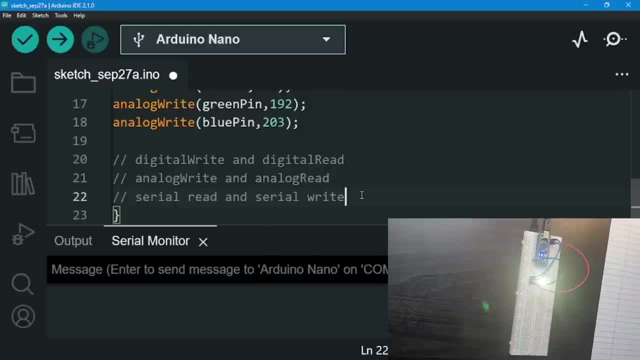 A serial write type of thing, because we're going to be what We're going to be: sending a message by using our serial monitor. Okay, So what's the idea here? The idea here is that we're going to set a color name right here. 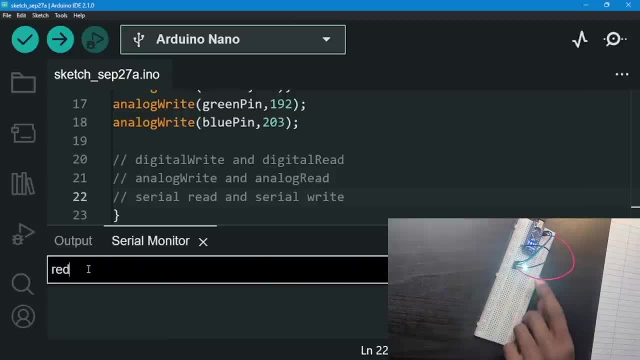 Let's say red, And what I wanted to do is I wanted to change this LED- the RGB LED, as I said, again capable of almost any color- to what To give me the equivalent color. So when I say red, I want it to turn to red. 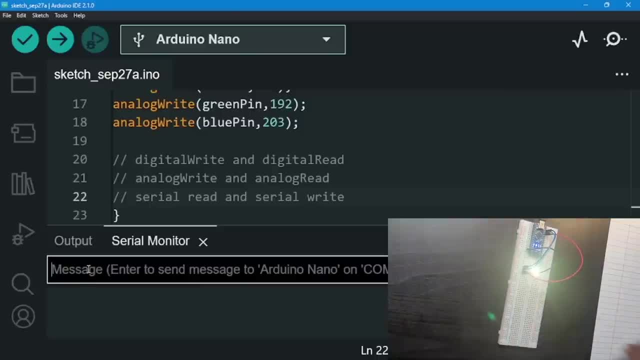 When I say blue, I want to enter blue. I want it to change to blue. When I say pink, I want it to change to pink. When I say purple, I want it to change to purple. Again, I want it to change to what? 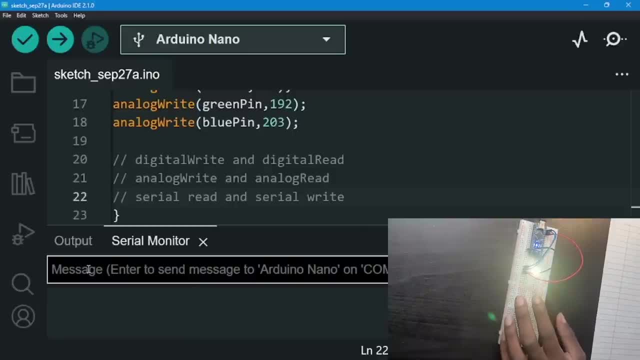 To the color. I already what That I set right here on the message. Okay, that's the idea of what we're going to be doing. So the question is: How do we even first receive the message from Arduino and how do we even code it so that what? 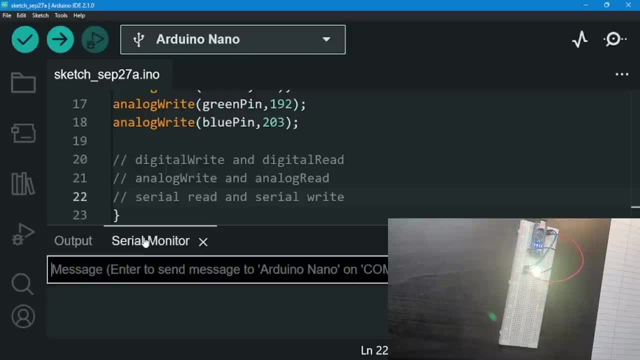 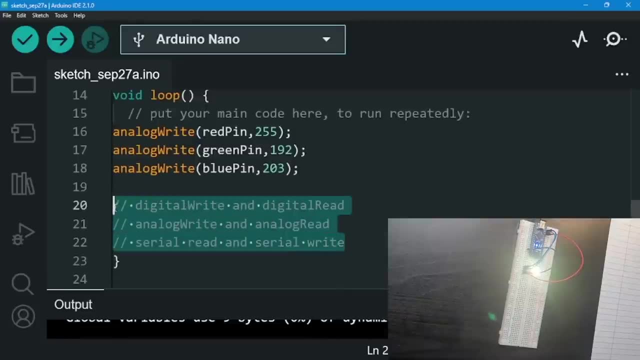 So that again, it gives me the equivalent color on the RGB LED. Okay, So let me just remove my serial monitor right now, And we're going to be working with it on the serial monitor. So one thing we need to do before working with any type of serial monitor is what: 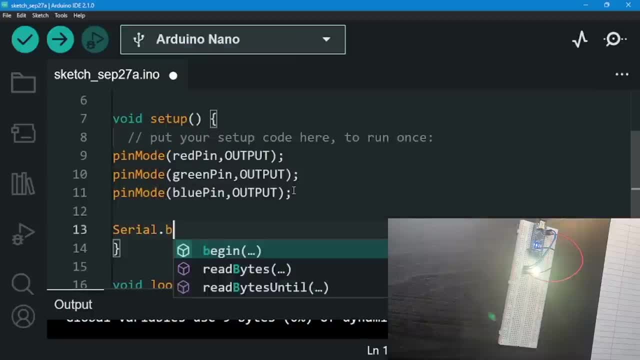 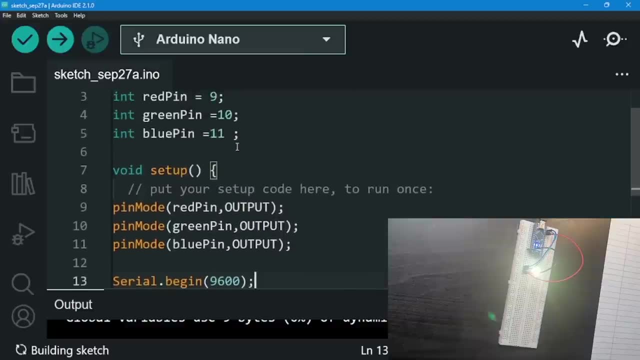 We're going to have to always what: Start our serial monitor. So we're going to say serialbegin and set it to what, To 9600, right now, And then we're going to be using, right here, serialreadString, We're going to be using something called what. 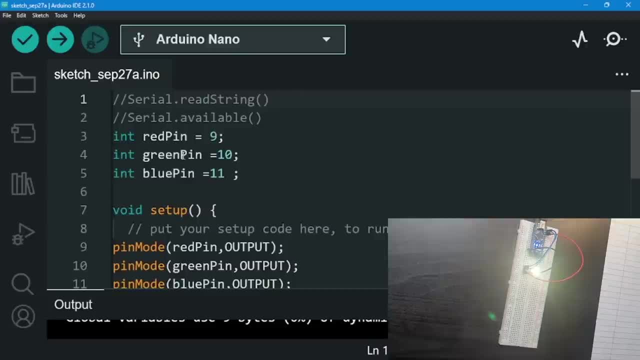 SerialreadString- Okay, So what I'm going to do right here? We already started our serial monitor right here. Okay, SerialwhatreadString. Let me just copy it. Okay, SerialreadString. There it is. So what does this do? 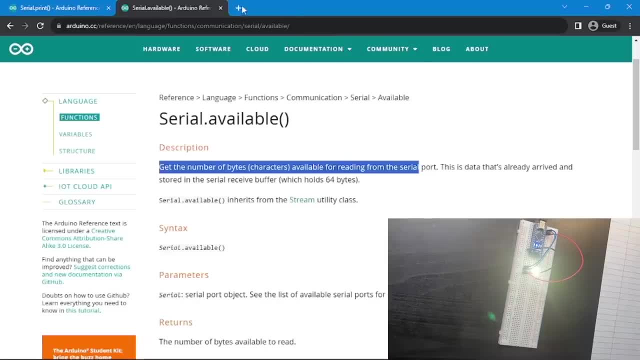 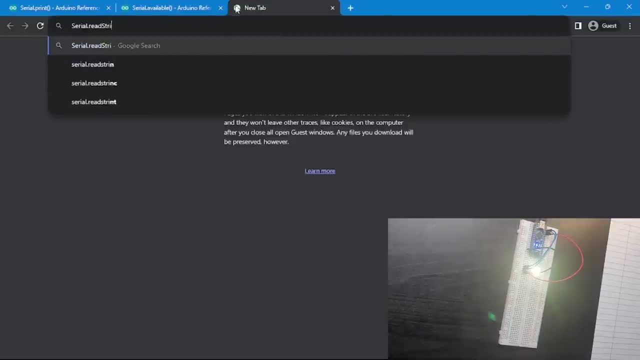 Let's just go to the documentation to check it for ourselves. So what does the serialreadString ReadString does for us? So let me just go to serialreadString And there we go. We have the Arduino documentation of it. There we go. 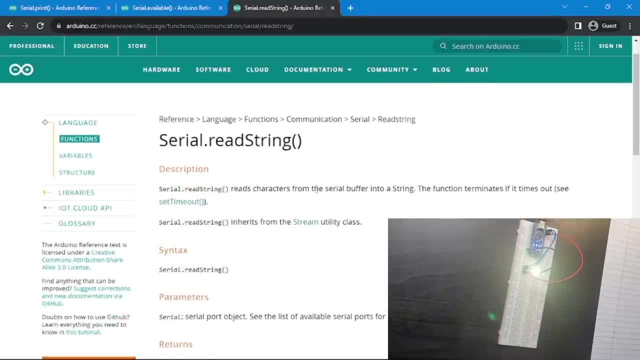 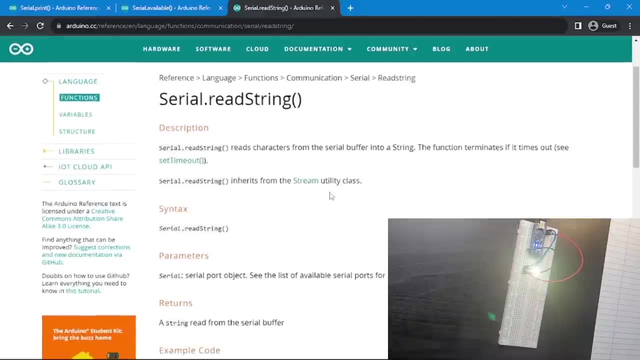 So it says: serialreadString reads characters from the serial buffer into a string. The function terminates if it times out, See timeout. So basically, what does it do? From a technical point? they say: what A serial buffer into a string. 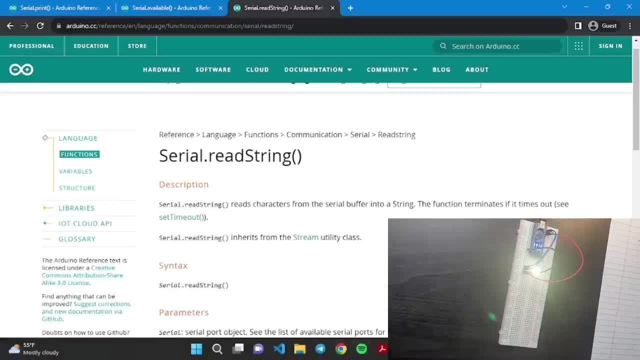 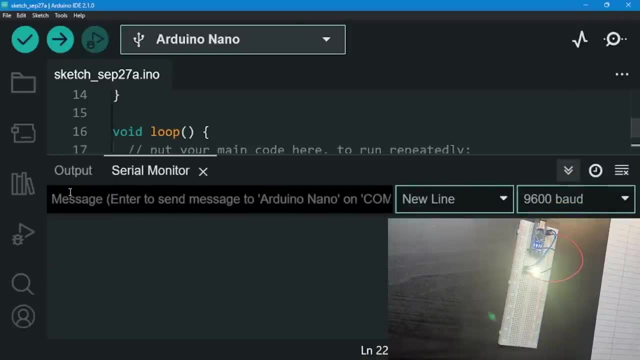 So, basically, what does it do is what It reads: the characters that are what Are going to be outputted right here. So it's going to be reading the characters that are going to be what That are going to be written on the message right here. 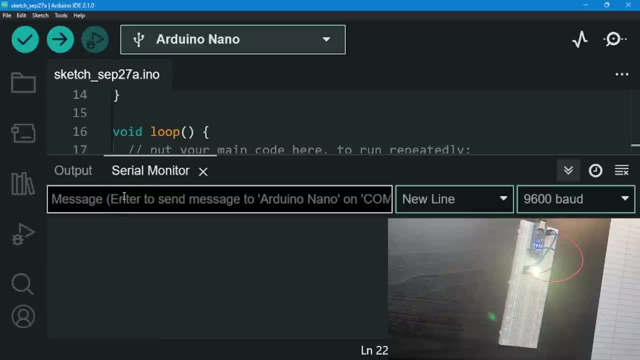 Can you see this? The message bar right here? This is the serial buffer And it's going to be what. It's going to be what, Reading the messages that are coming from here. So we're going to be using what? 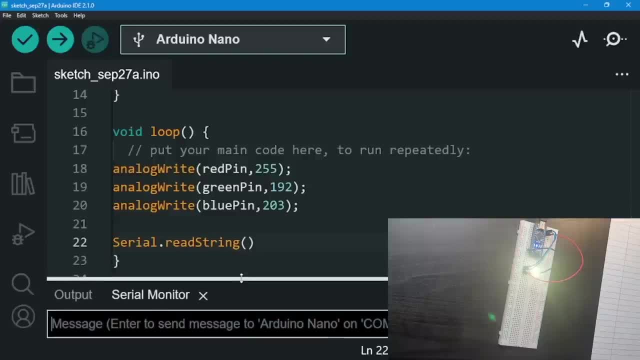 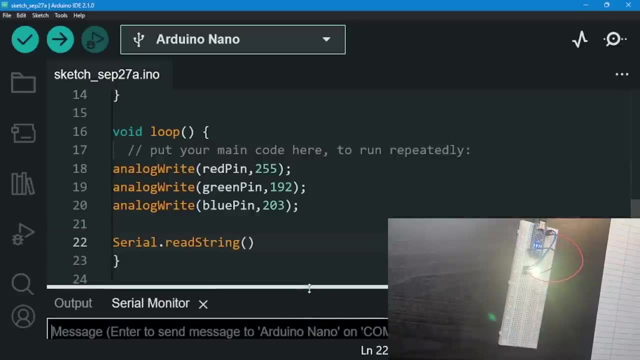 SerialreadString to what To read messages that are coming from, what That are coming from our message bar right here, or our serial buffer. Okay, So, right here. what we're going to do right here is we're going to need a new value, a new variable. 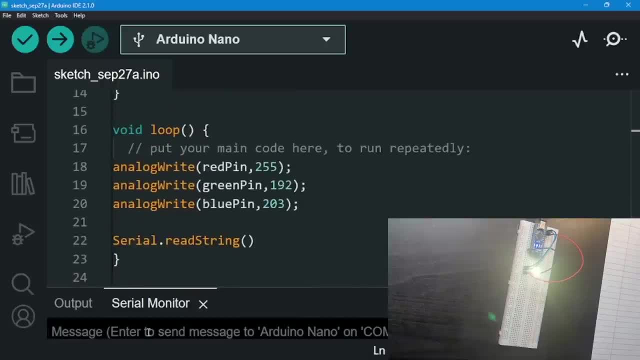 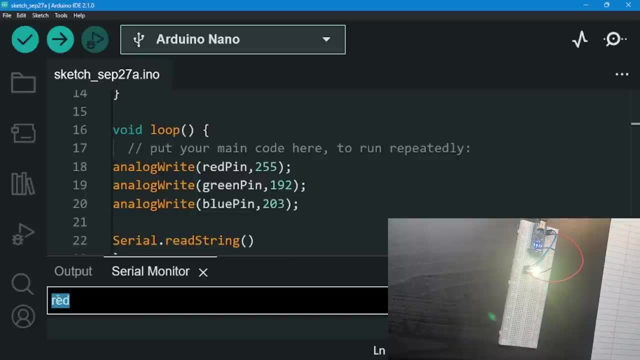 We want a what. Once we get the value, let's say, right here, I have red, I put red right here. Let's say I put red, right here, I want to what. I want to store it because we're going to be using it in our code. 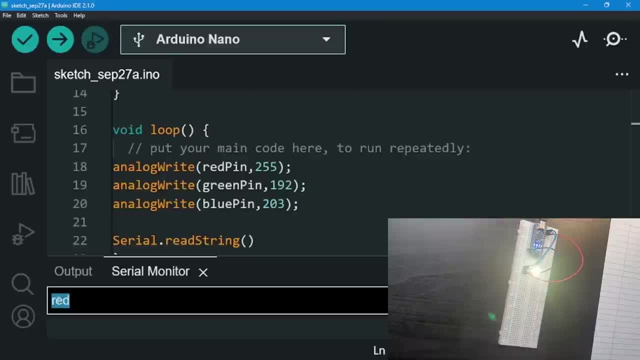 So what? So I'm going to be using it later in our code. So what? I want to store it in a what? In a variable, Okay, So let me just do that. So what do I need right here? 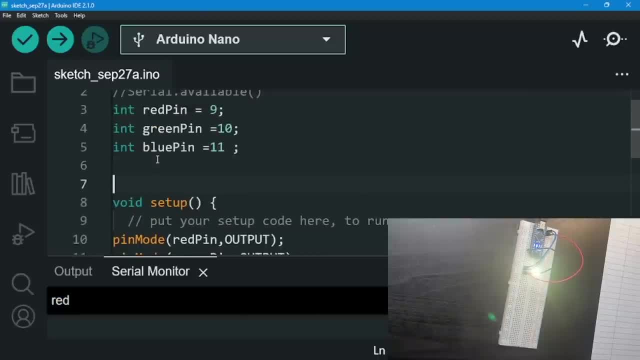 I need a variable. So what is it going to be right here? What type of variable is it going to be? Am I going to say integer? Am I going to say you know what? This is going to be the set color. 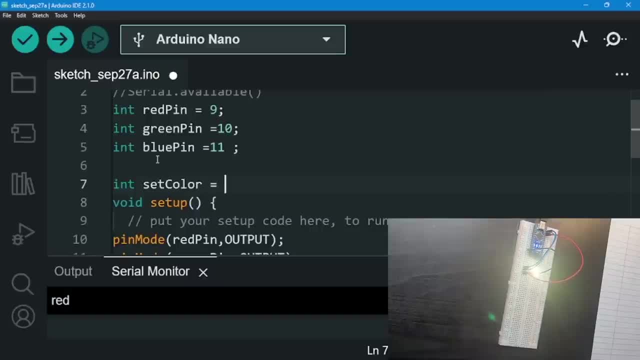 Let me just say set color right here. Set color. Is it going to be integer? Is it going to be an integer when I set it up? No, What is it going to be? A string? Okay, A string. Am I correct? even how to write it down? 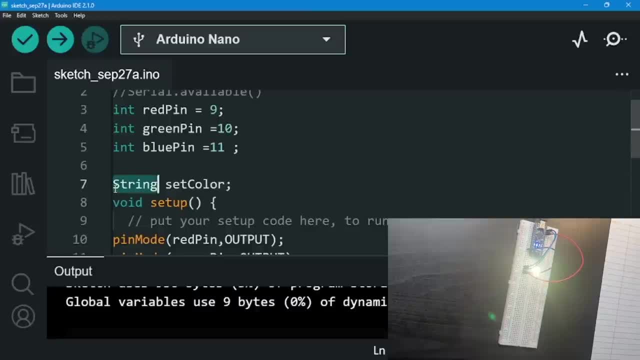 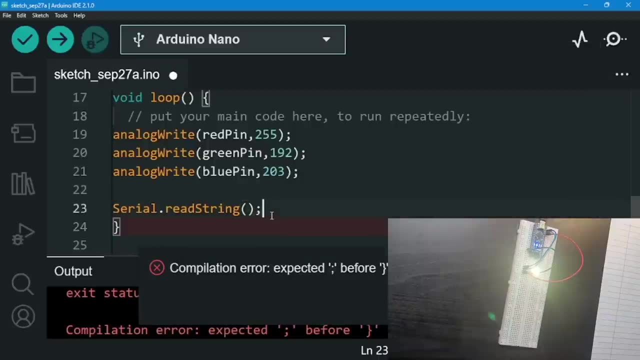 I think it's string. Let me just again to always check that everything is correct right here, let me just try to compile it. saying that it expected a what? Oh, It's a semicolon. Let me just compile it, Okay. 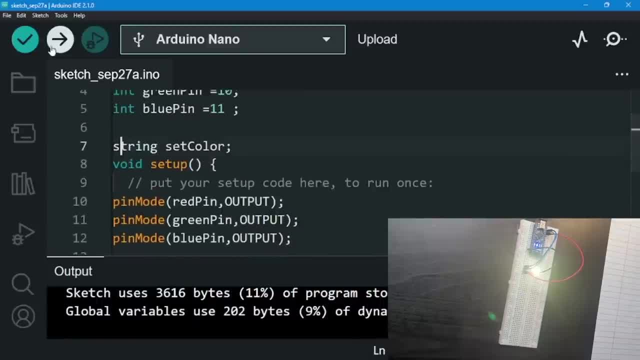 The capital S is the right one. If I put a small s, Well, let's see what happens if I put a small s right here. Okay, There we go. Let's say it's an error. I have to say capital S. 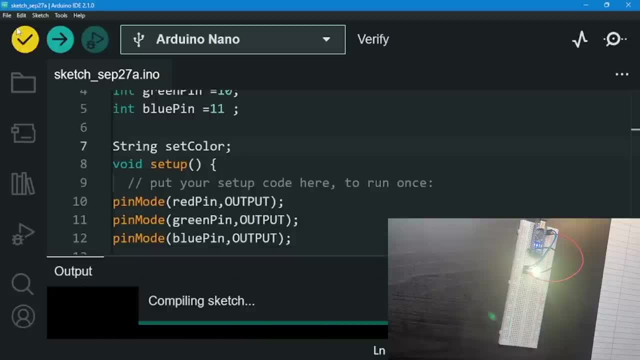 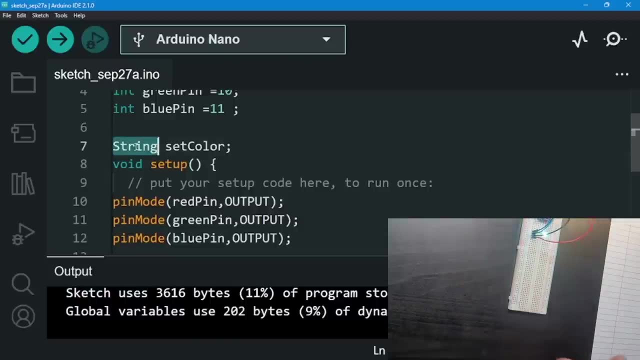 Capital S is the right way of writing it. Okay, There we go. So you might be wondering what is a string? Let me just go over this so that it becomes as simple as possible. Okay, So a string is right here. 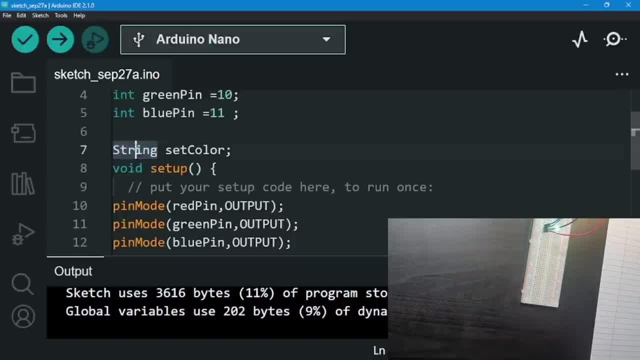 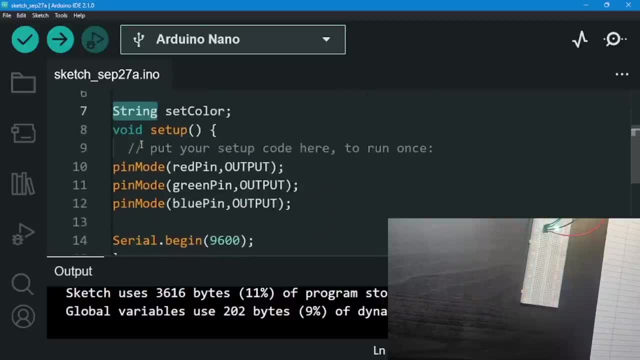 I'm not going to use my paper. actually, I think it's better to use my screen. So, right here, what does a string mean? Okay, A string means a normal text. Okay, For example, this is a normal text. right here. 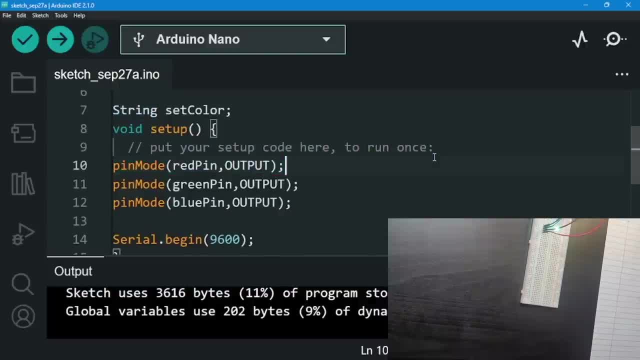 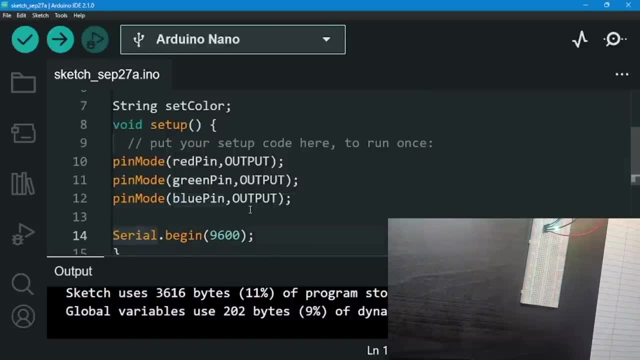 It says: put your setup code here to run once. Okay, But right here, pin mode is what? Pin mode is a what? Let's go right here. Let's use an example of pin mode. What is pin mode right here? Let me just go to pin mode. 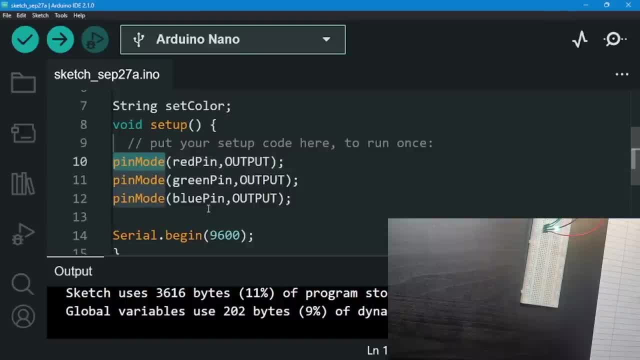 What is pin mode? Pin mode is a what. It's a command. It's a what. It's a code. Okay, It's a code to be what Executed. So one thing it wants to identify is what It wants to differentiate between a normal text and a what. 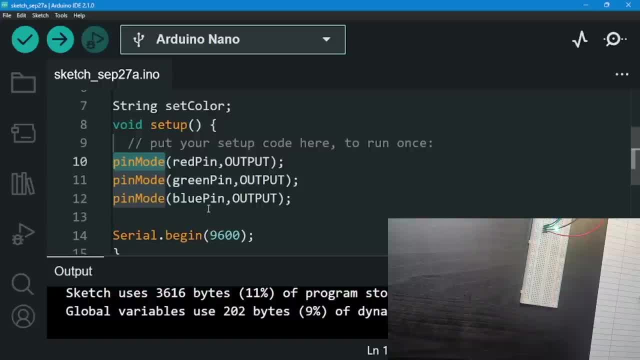 And a what, And a normal what And a normal code. So it wants to differentiate between what Code and text, Which one is text and which one is code. Because if we don't do that, we're going to get into what. 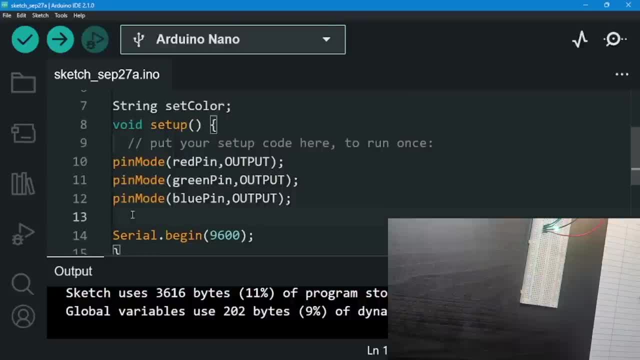 We're going to get into lots of troubles, Because if I just say right here, instead of let's say I'm just saying hello world, it's going to expect let me just say hello world. right here, Okay, Let me say hello world. 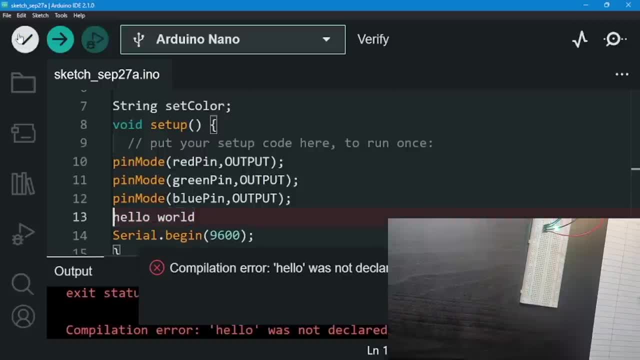 Okay, Let me just try to compile this, Let me verify this. Look what happens. Hello was just not declared in the scope. It's trying to find what It's trying to find a command, a code named hello world. Okay, 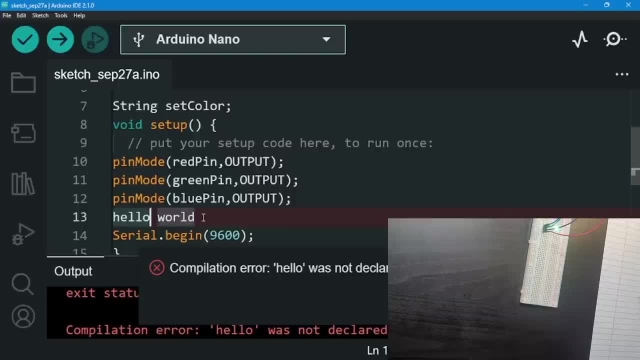 It's trying to find what A code named hello world. Obviously, there's nothing called hello world in the Arduino. Obviously that makes no sense. So what it basically means is what It does not understand: that it's a normal text or a code. 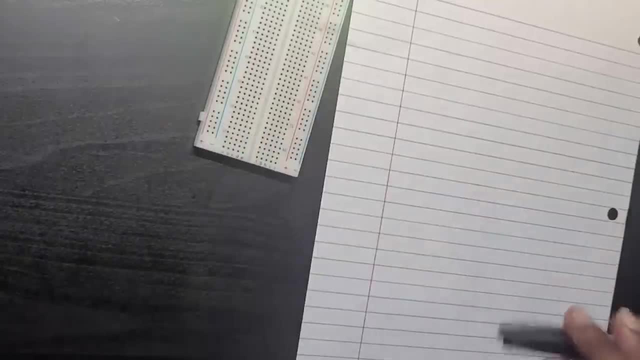 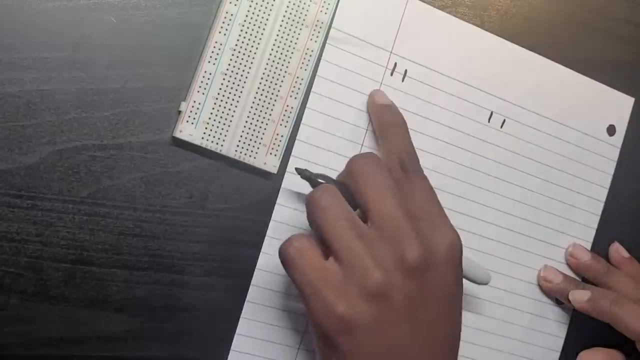 So to differentiate that, we use what symbol We use right here, What do you use to call it A quotation mark? You see that A quotation mark. So we use quotation marks right here to what? To identify a one. that is what. 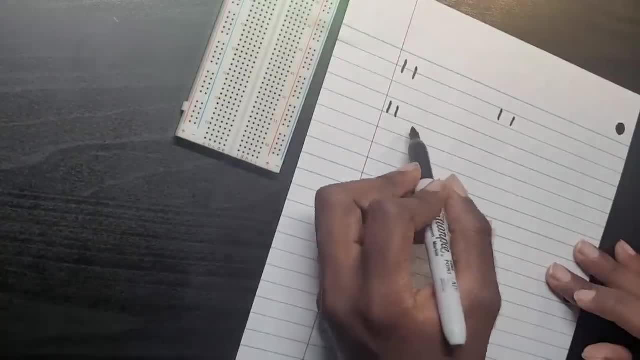 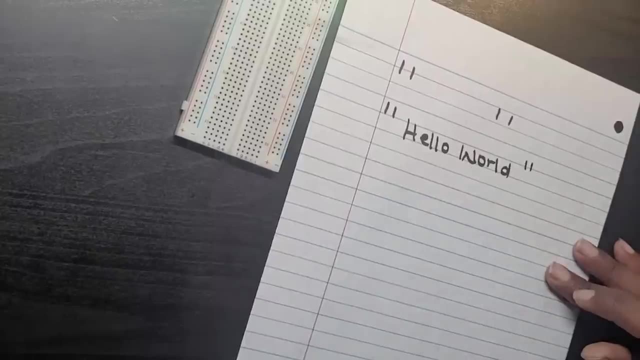 A code and a string. So in strings we say double mark right here And let's say hello right here, Hello world. If I say that it's going to what Render it as text, It's going to treat it as a what? 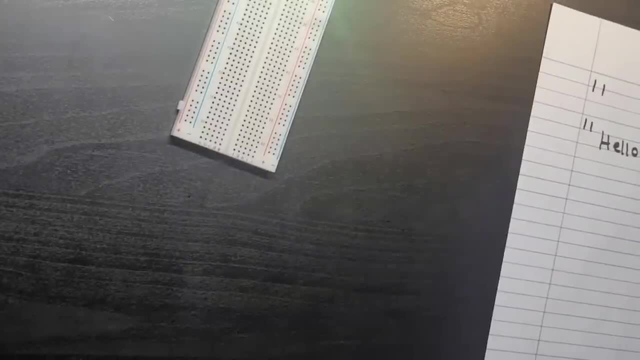 As a normal text, So it's not going to be giving me an error. So let's see what happens. if I just say: you know what? There's a string, It's a name, Just say hello world, Okay. 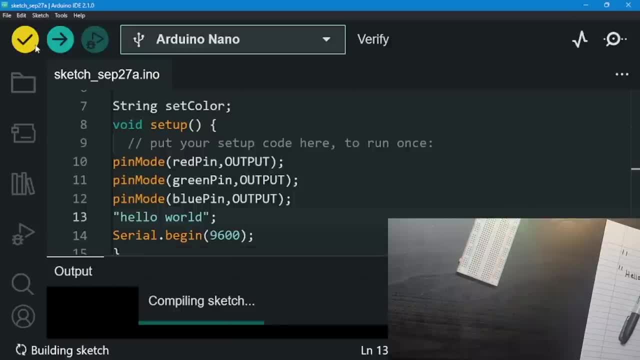 Always finish it with a semicolon right here. How about if I upload it right now? Let's see what happens. It's done compiling. You see that It's done compiling. It's not giving me an error, It's saying as what? 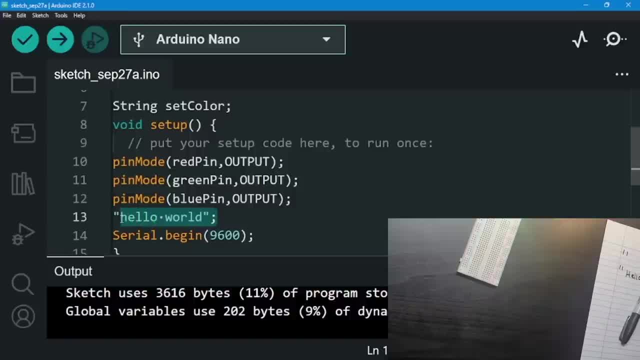 This is just a normal text. Don't get into what. Don't get into detail, Just write what. Render it as a normal text. Okay, Don't do anything further than that. It's not a command, It's just basically what it's telling it. 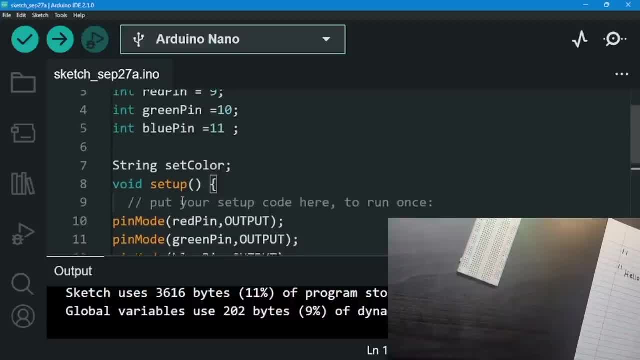 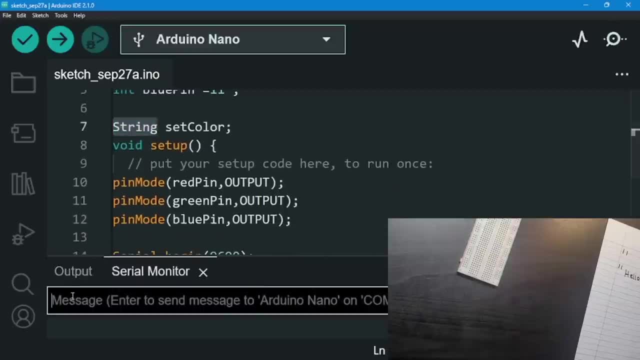 So what? It's a normal text. So Right here, Basically, what are they called? They're called strings. Okay, So keep that in mind. Because, why? Because I said again, we're going to be working with what. 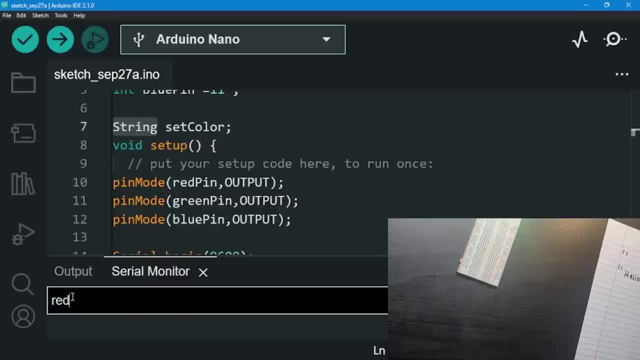 With what? With letters right here, And I wanted to render it as what. It's not going to be rendering what. It's not going to be searching for the what For the command or for the code red. It's going to be searching for what. 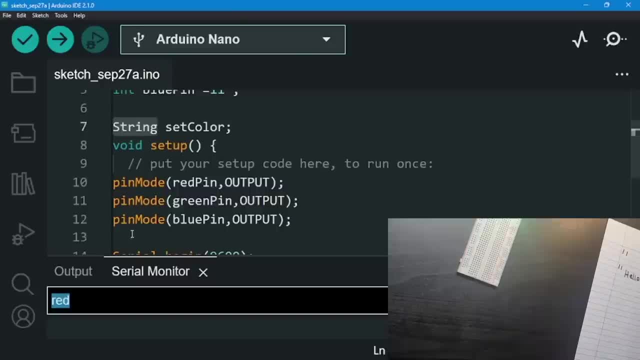 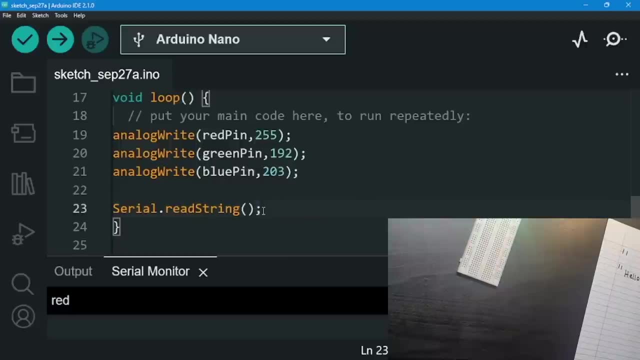 It's going to be searching for what The string red. It's going to make more sense as I go, Okay, So right here, I wanted to what To read the string. How do we set this? Once it meets the string, I want to set it to what? 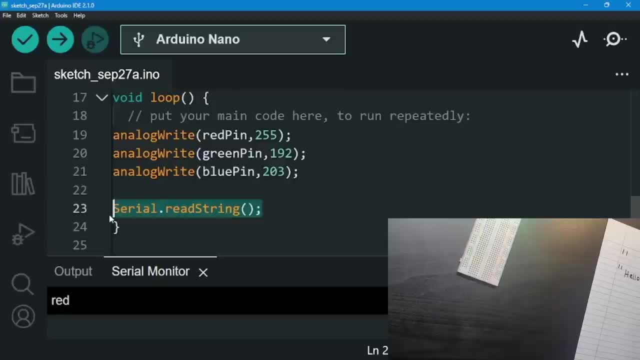 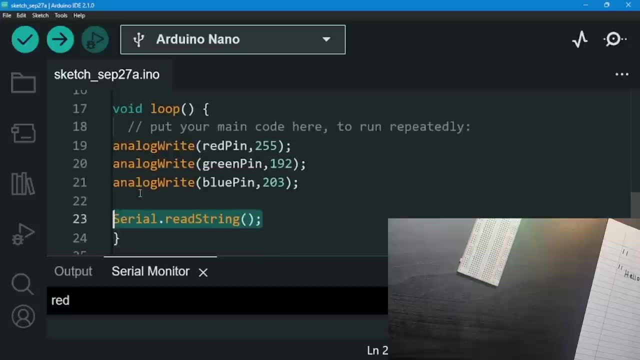 To a variable? Okay, Because why I want to what? I want to use it for what? For later purposes. So how do I do that? What I do is I go right here Set color. I say set color. 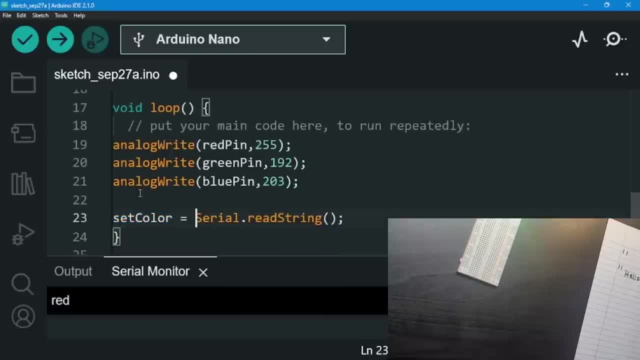 Let's go right here, See set color. Set to what Set color is equal to the string red value. So once the value is read right here, as soon as Arduino reads the value, as soon as, let's say, I enter a value right here, and it reads it. 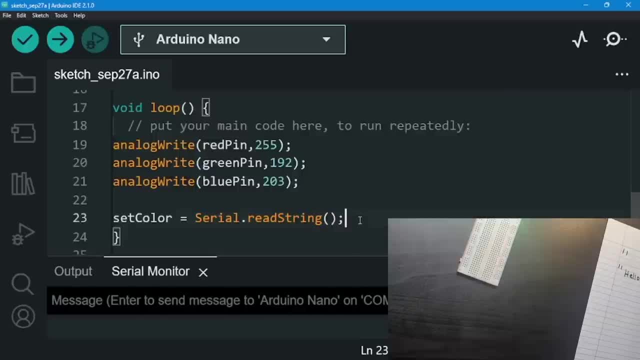 it's going to set it to what? It's going to set it to red, right here. Okay, It's going to set it to a value, The string that we just wanted. That we just what. That we just read right here. 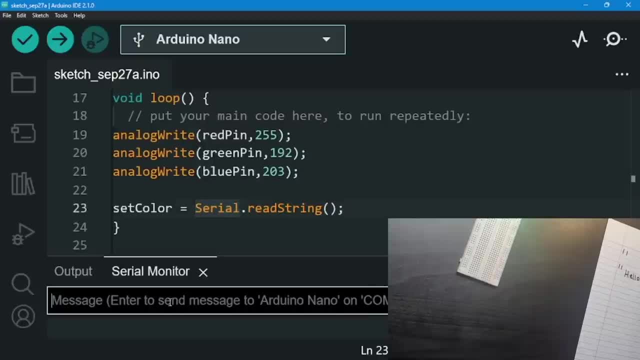 Okay. So what does this mean? So, for example, if I said read, right here, I just say read and enter it, what is going to happen? Set color, Set color is going to be what. Go right here, Set color is going to be what. 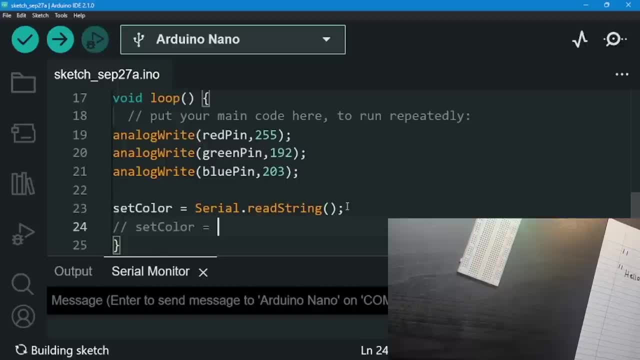 Set color is going to be equal to what. It's going to be equal to the string: red. Again. what is one thing we have to acknowledge? What is it? What is one thing that we have to acknowledge? This is what A string. 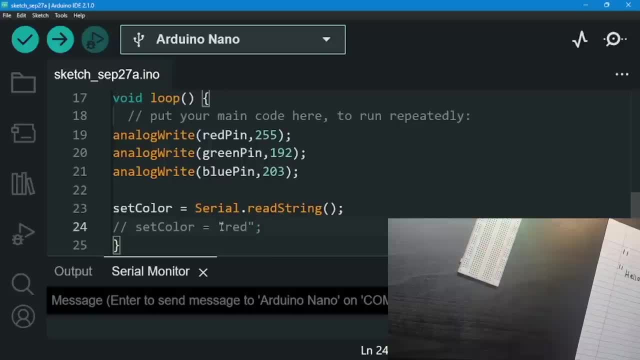 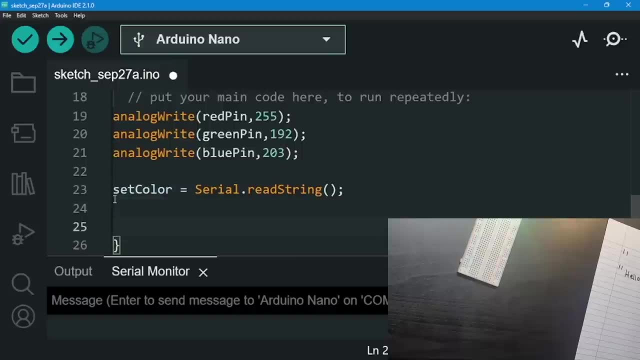 There's what The quotation mark is right here. Okay, Keep that in mind. Okay, So, with that in mind, now what we want to do is we don't reset the color, Okay, So let's try to print what we just wrote right here. 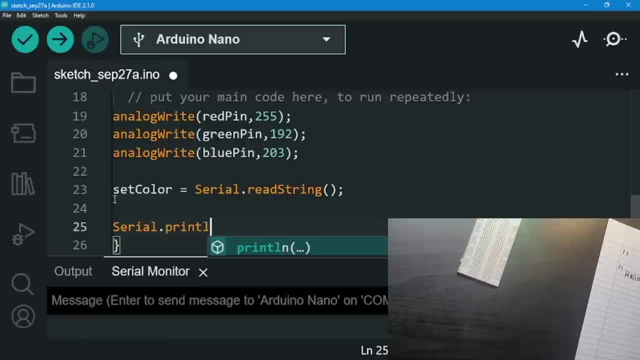 So to actually see if it's working or not, let's just print it. Okay, We're going to say println and say set color. I just want to print it so that let's even see if it's what It's rendering, the right thing. 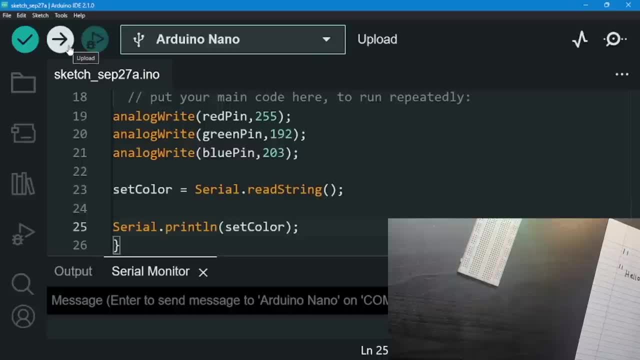 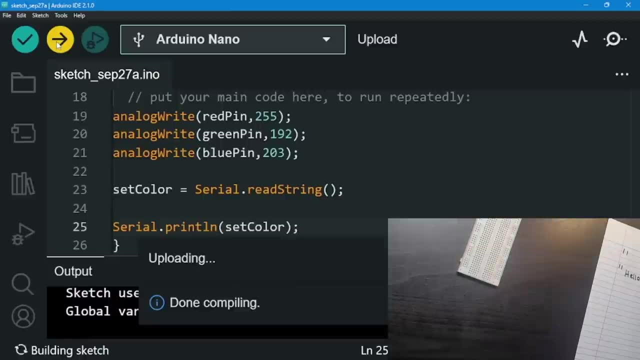 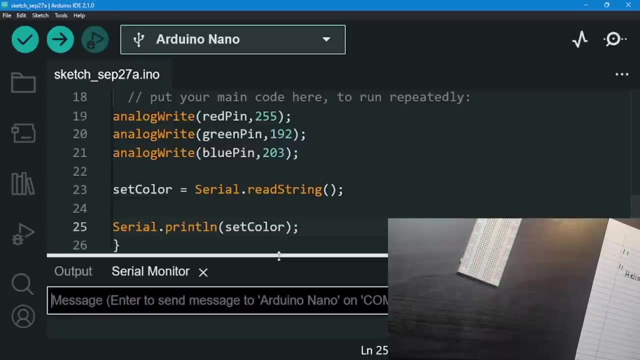 Okay, So let me just upload this. But before doing what should I do? Turn off my serial monitor. Hit that And now I can upload. It's done compiling and it should be done uploading. Okay, So let's go back to our serial monitor right here. 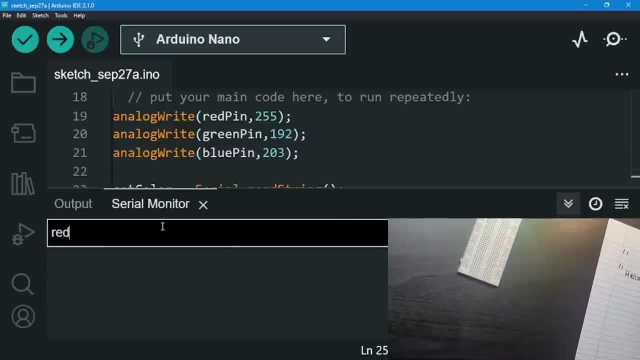 Let me extend it a bit so you can see it better, And let's try to say: red right here. Does it print red? There we go. It printed what Printed red. Can you see that It printed red? And you can see that it's printing out empty stuff. 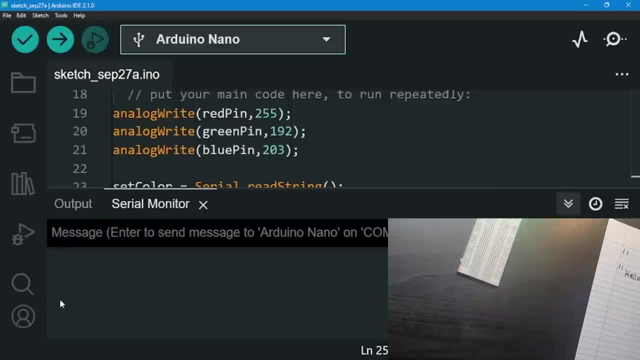 Can you see that It's printing out empty. What is it? What is going on? You might be wondering what is going on? Okay, What is going on? You might be wondering: why are we printing out after red? We're printing out something, something. 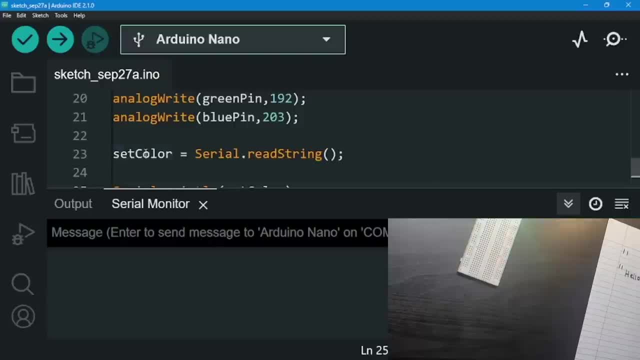 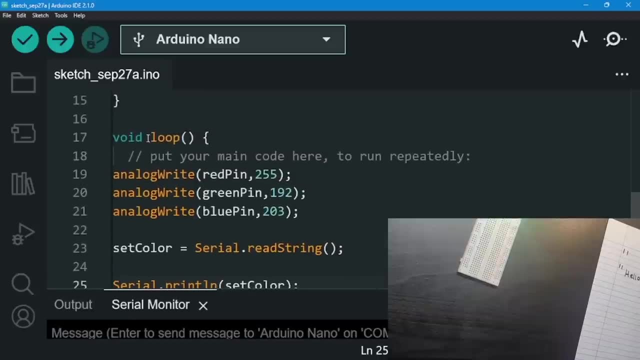 What are we printing? Some empty spaces, some empty stuffs. Why is that so? Let's see what happens Again. one thing again you have to keep in mind is what. One thing you have to keep in mind is what It's going in a loop. 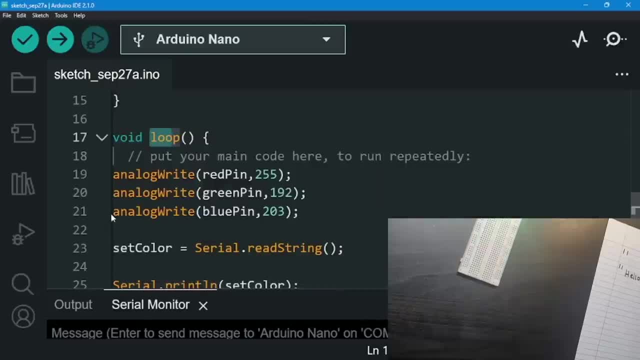 So it's going to read it one time and it's going to be, you know, setting the analog right to again all these values Afterwards. what does it do? It reads the string. In this case it was red. 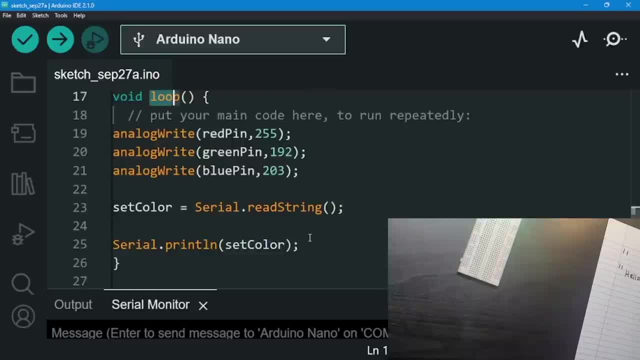 I already wrote down red. It's going to set the color. As I said again, it's going to what Set the color. So basically what, Sorry, I said set color. It's going to print it out. It's going to print the what. 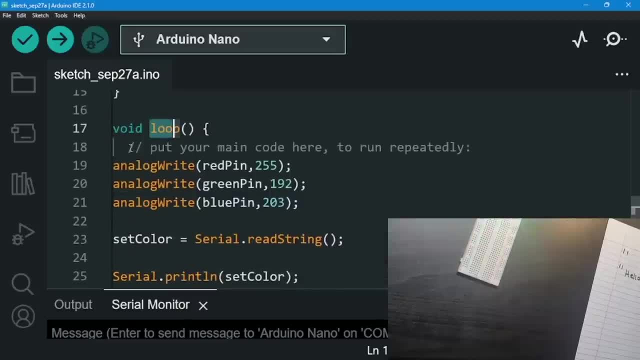 The variable set color, And then what happens? And then it runs it again, But this time I have to write it what I did not write it this time, So it's going to start from again. It's going to start from again, as I said. 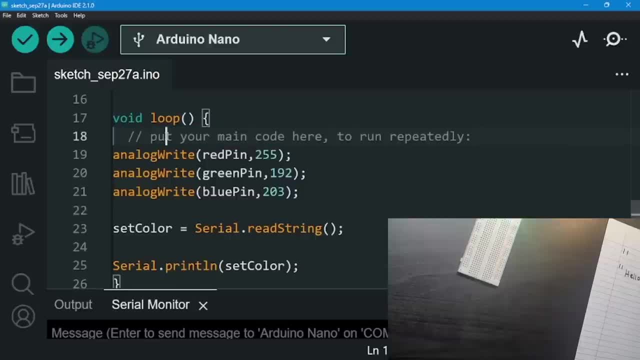 It's going to start again because this goes in a loop. again. It's going to start again. Do the same thing, but right here. What happens here on the read string? In this case, what did I do? I did not write down red again. 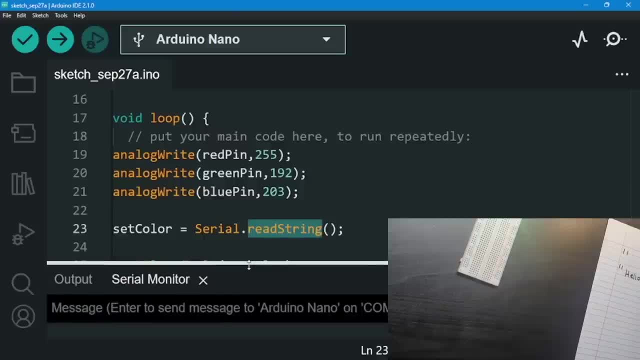 I have to write down red at very, very fast speed for me to what To match up to what To match up to the Arduino Right here. what's going on? The read string is what? It's: an empty set, because I did nothing. 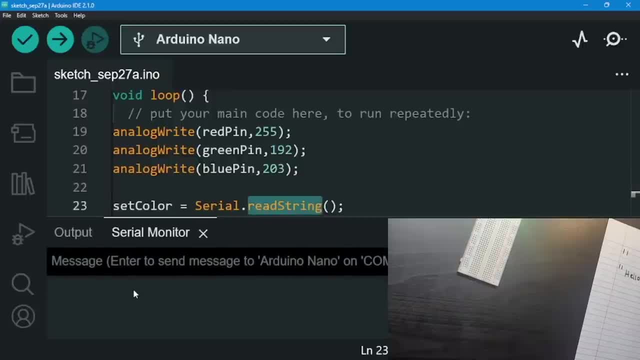 It's basically what? It's basically empty because I did not enter anything, So it's going to be giving me those empty spaces right here. It's printing it out. You can see that it's printing out what Empty spaces. Okay. 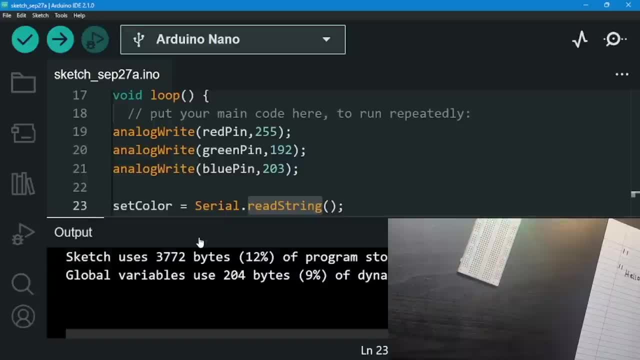 So I just want you to keep that in mind. Okay, So right here, it's going to be printing out this, We're going to fix this, And then, by using space, we're going to be using something called SerialAffailable. 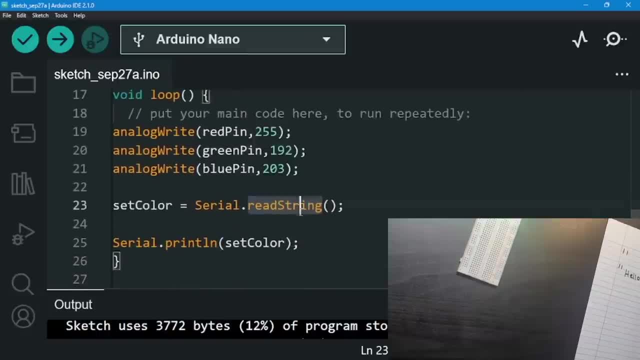 I'm going to get to it, But now let's focus on just optimizing the read string. We're going to go back and fix this later, Okay, So right here, let me just forget about the printing. It works, But obviously what happens again. 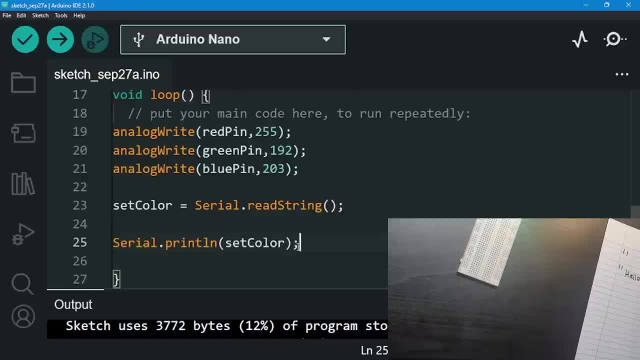 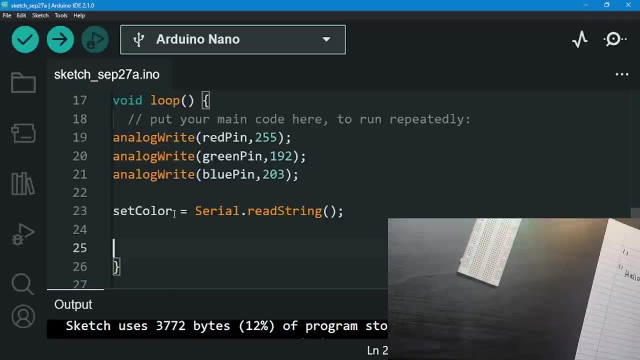 The problem here is what It's going to print out those empty characters. We're going to fix that on the next one, Okay, So one thing we want to do afterwards, after we store our set color, is what. Our set color is what. 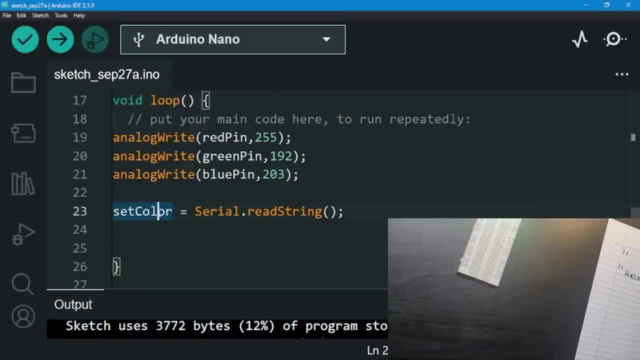 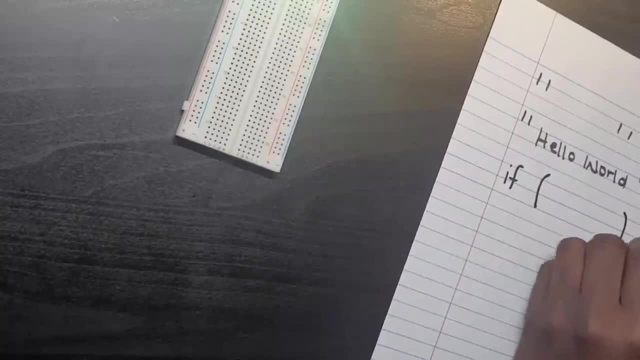 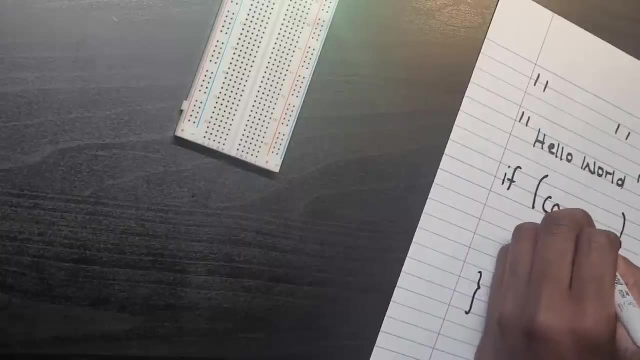 We want to compare it, Okay, So how do we do that? So right here let me write down an if condition. There's the keyword called if. Okay, We have curly brackets. right here. Our condition is written inside here. 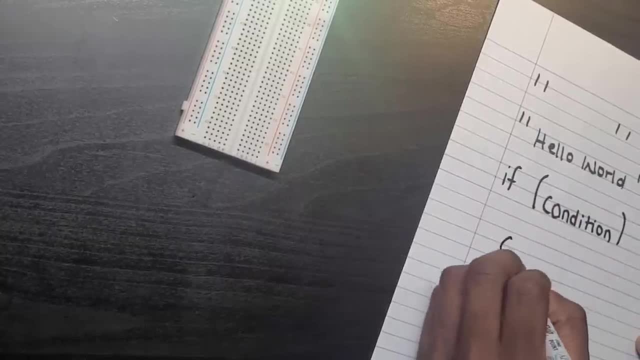 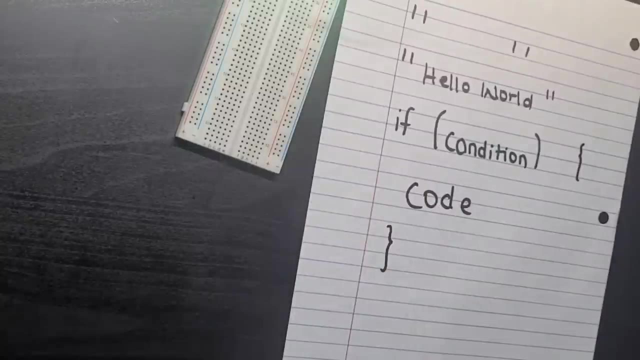 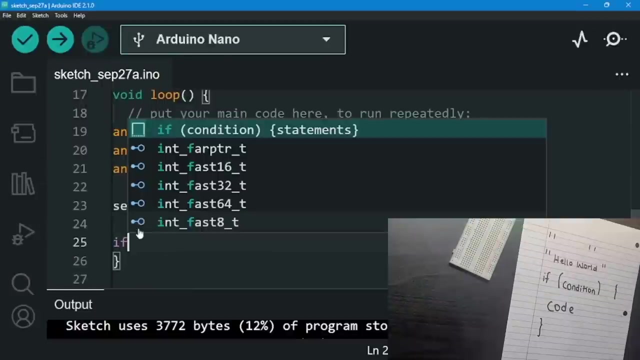 Okay, Our condition, And then our code is going to be written inside of the curly brackets. Okay, So, when it comes towards these if things, if you write them down, let me just write them down right here. If I say if it has what, 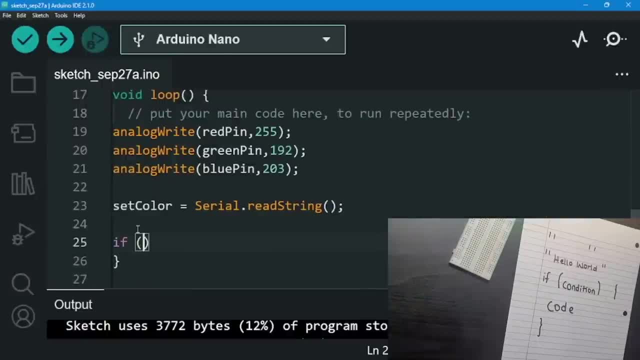 A special color. Okay, It's a code. as I said again, We're going to write down our condition, what- In those curly brackets, And then we're going to have our code in the middle of those what's. 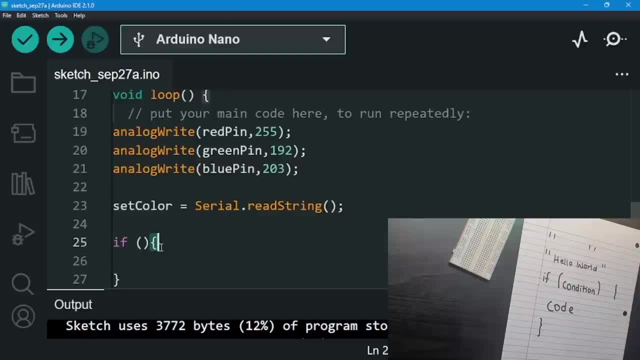 In the middle of this, what Curly brackets again. Okay, So this, what This quiggly brackets right here, Okay, So in the middle of this, sorry, the what In the middle of the curly brackets, Sorry. 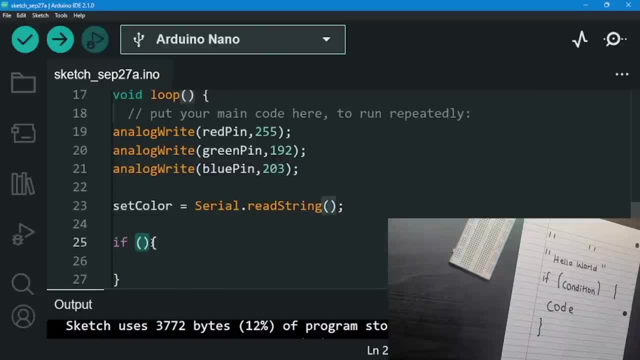 I keep saying curly brackets for this one. This is called a parentheses. Okay, In the middle of this is going to be the condition. I got that wrong when I said it, But in the middle of the curly brackets is going to be our what. 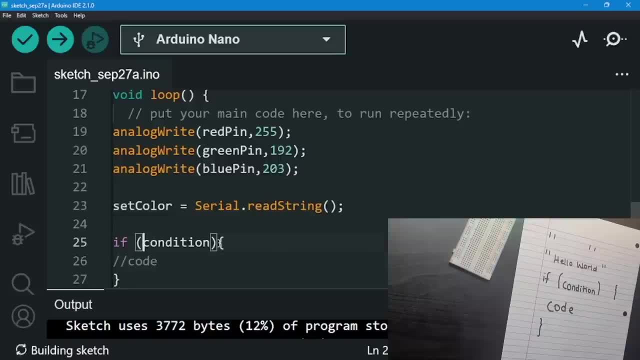 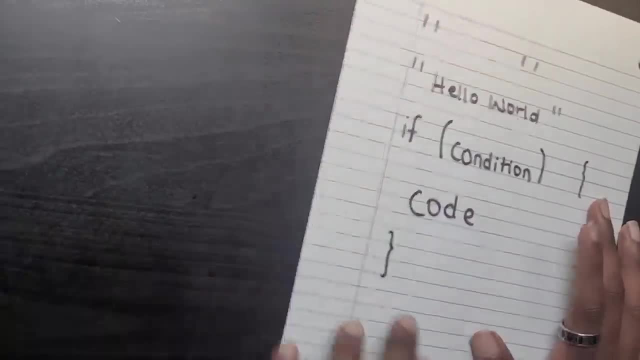 Our code. It's going to be written here, Okay. So one thing I want you guys to keep in mind is: let's use a very, very simple analogy so you guys understand this. So I think most of us have obviously had this English lesson about what? 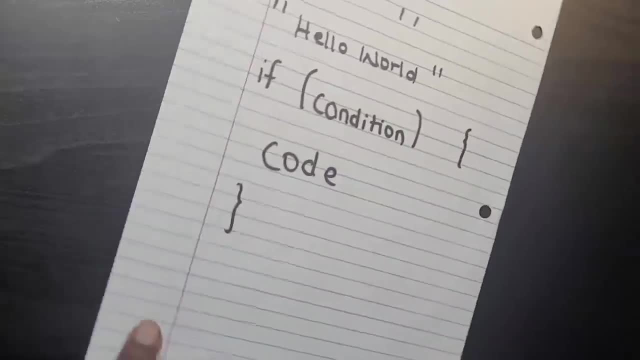 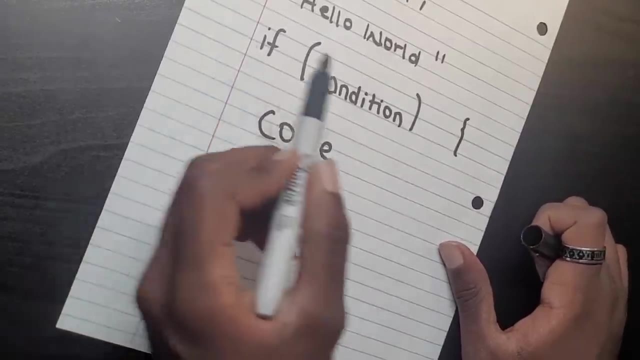 If condition tenses, condition tenses, if you remember. So, when we learned about condition tenses, what did we say? What did we say? There's a condition, There's if and there's a condition. and then there's what. 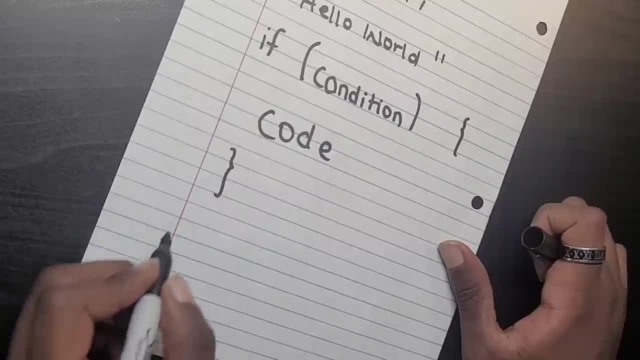 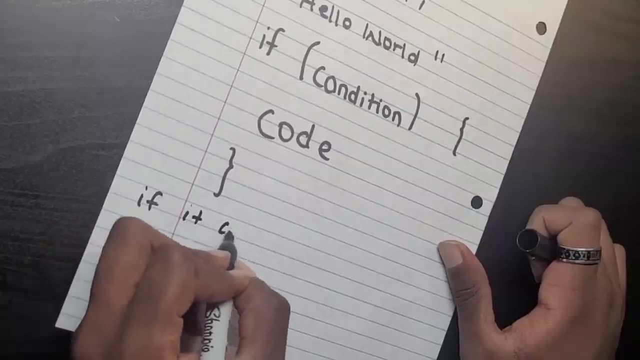 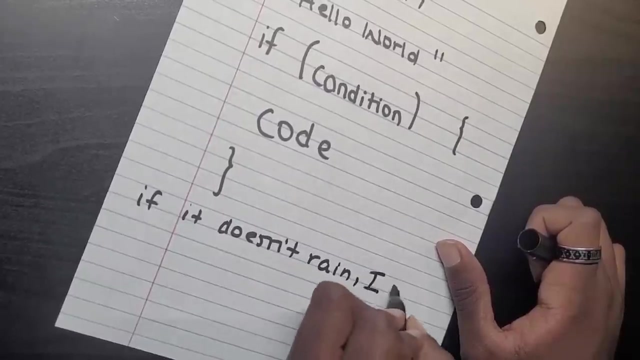 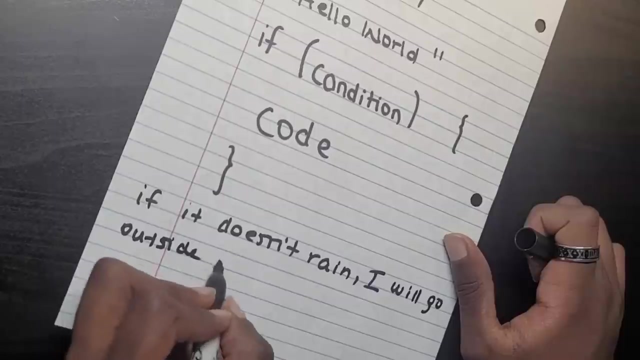 And there's what And there's the result of that condition. So it's like cause and effect. So one good example would be: if, Okay, If it doesn't rain, if it doesn't rain, I'm going to say I will go outside to play basketball. 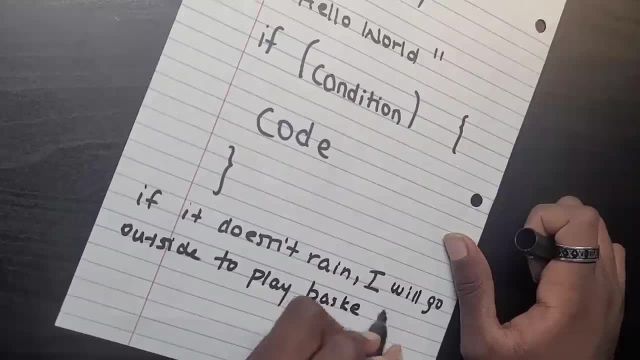 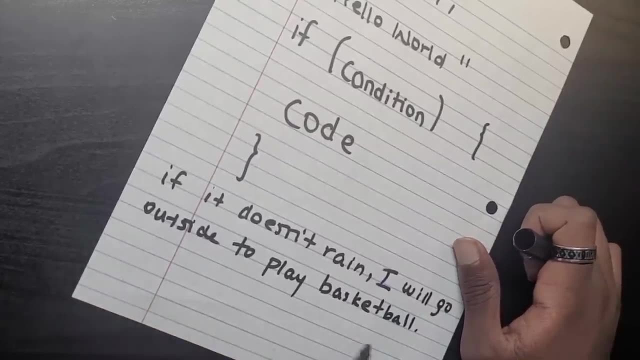 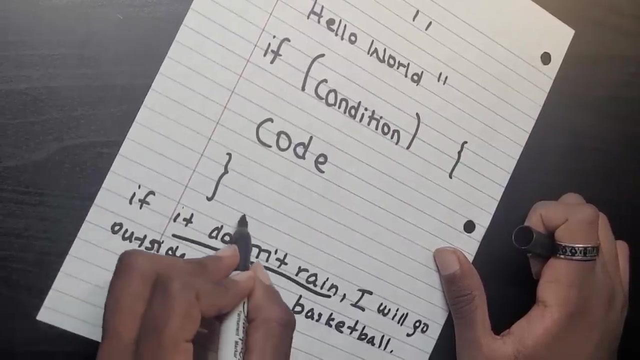 Basketball. Let's start to analyze this. So, if it doesn't rain, I will go outside to play basketball. What is the condition here? The condition is what It doesn't rain is what The condition. This is what Our condition. 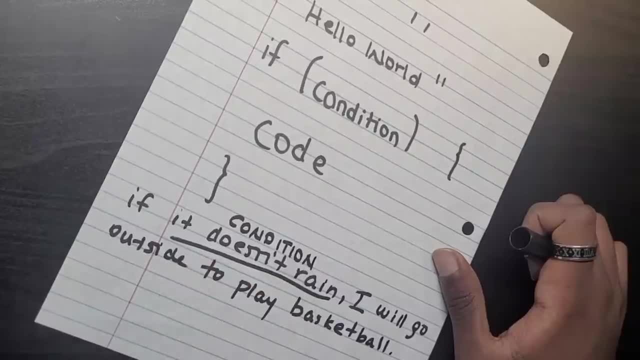 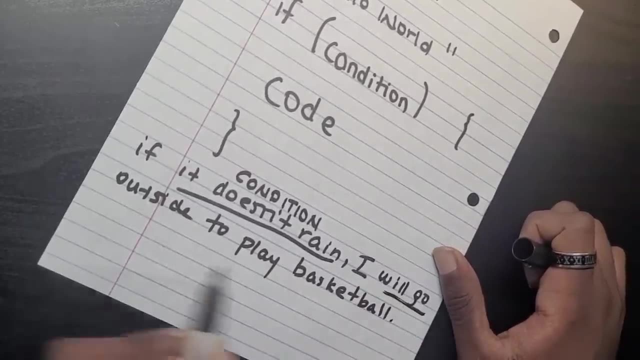 Okay, this is our condition And the result of the condition. again, the consequence of the condition will be: what, What I? what will go outside There, What That To play what Basketball. This is what This is going to be our action, basically. 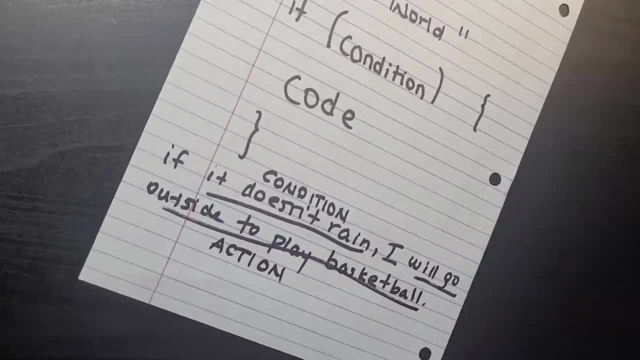 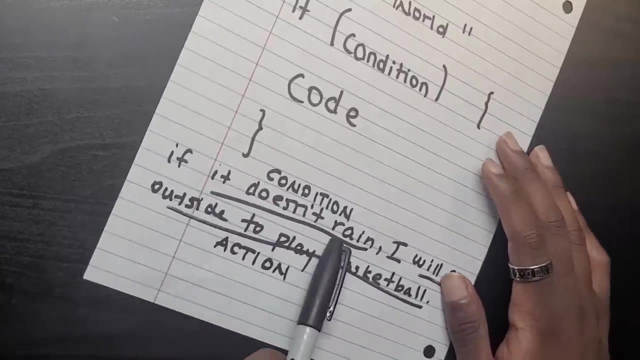 Action. So there are two things to this condition. again, There are going to be what? Two cases to this condition. What is that? What are the two cases In this case? one case is what: It doesn't rain, So what? I can just go outside and play basketball. But there's another condition too. 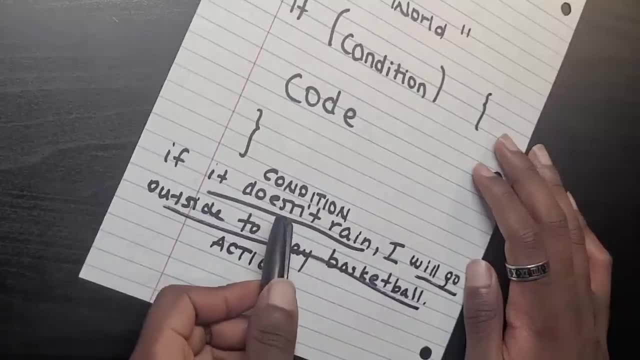 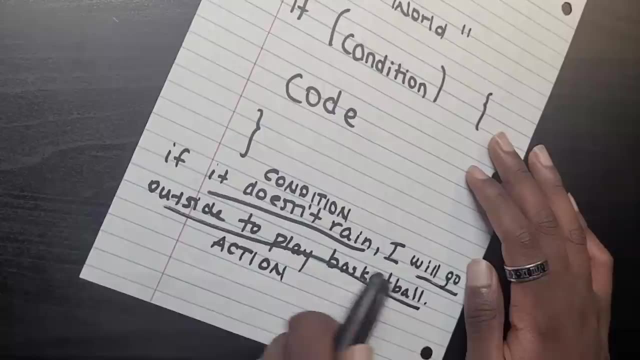 When this condition is false, basically When it's what It's raining. When this condition is not satisfied, it's raining outside. basically right now, What is going to happen? I'm not going to go outside to play basketball. I'm not going to go outside to play basketball because I don't. 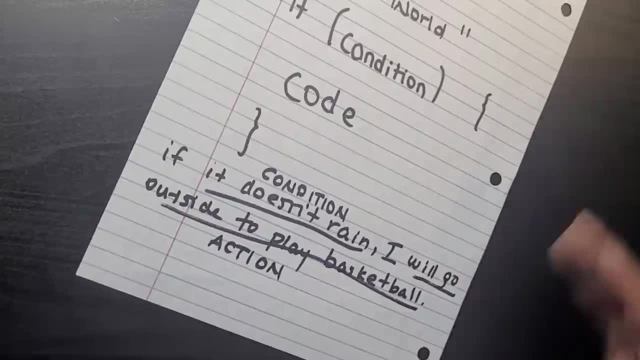 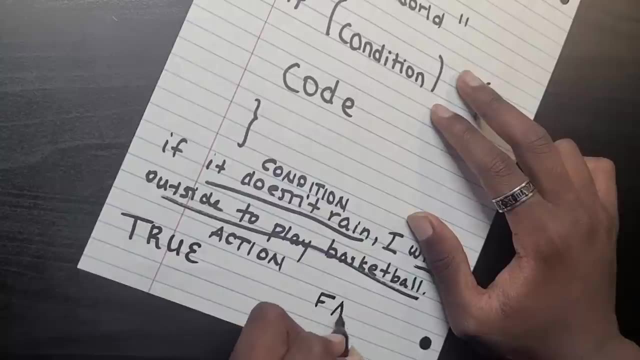 want to get wet. Okay, I just want you guys to keep that in mind. So when this condition is what It can be said to true or what It can be false, Okay, Both of them will have what When it's true. 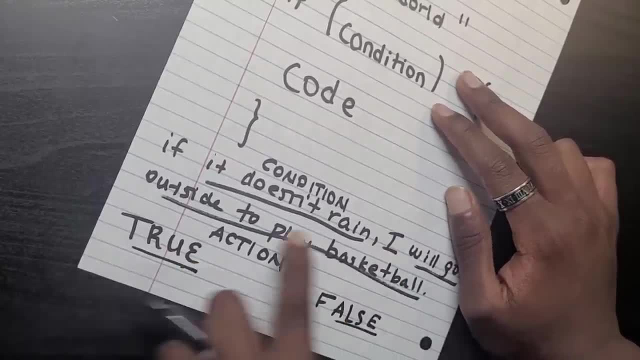 it's going to have what. When it's true, it's going to have what. I'm going to go and what- Play basketball. When it's false, in this case, what It rains, What am I going to do? I'm. 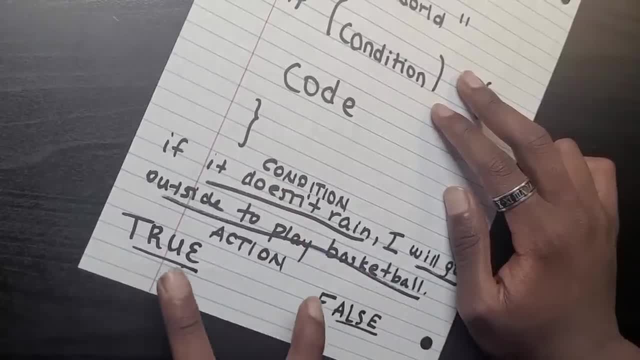 not going to go and play basketball. So it's going to have what? Two scenarios: When it's what, When it's true or false, When the condition is what, True or false. So it's going to have what? Two again cases, as I said again, Okay, So it's going to what Affect our, what, Our action Again. 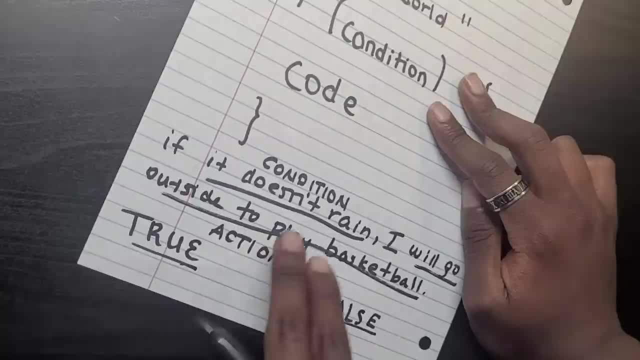 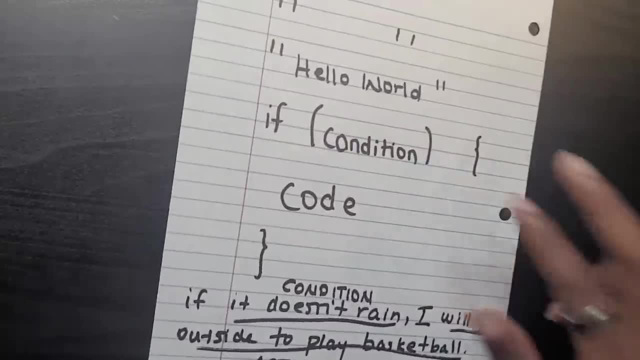 it's going to affect our action. This condition is going to affect our action. The condition coming true is going to affect our action And the condition coming false is going to have what Another effect in our action? That's one thing I want you guys to keep in mind. So it's going to. 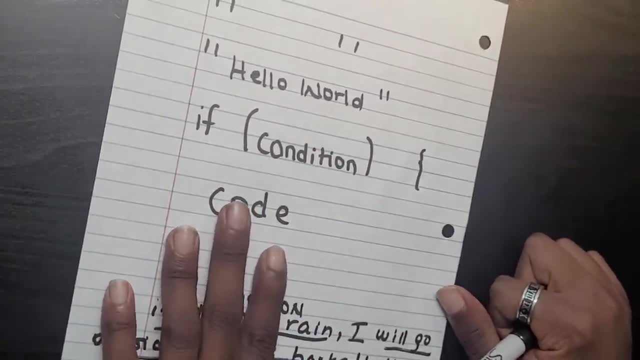 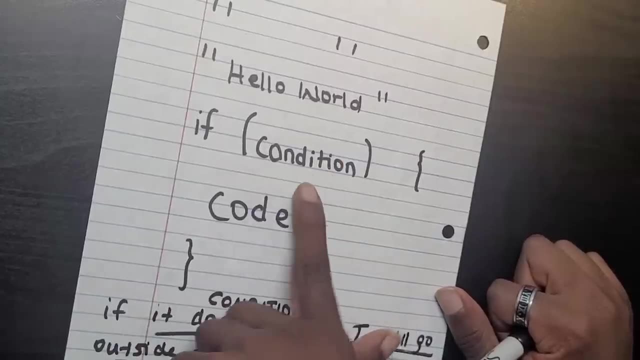 be the same thing, too when it comes to computers. Okay, So what? There's an if right here and there is a condition. We have a specific what. We have a specific condition, And then what? When that condition is satisfied, what's going to? 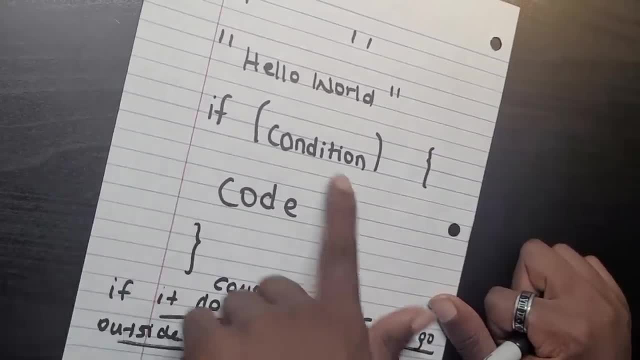 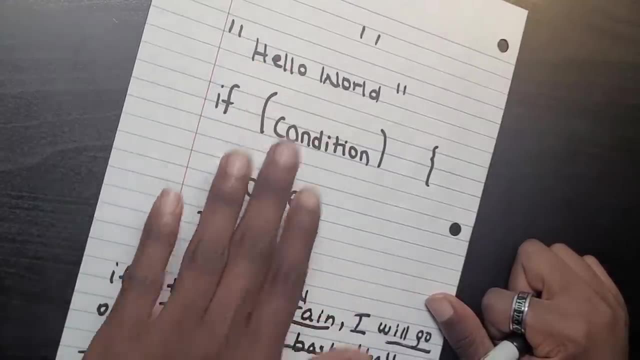 happen. It's going to specifically what It's going to, what It's going to execute the code. that's here, Okay, When the condition is not satisfied. it's going to what It's going to skip it. It's going to skip what, The whole, what, The whole bracket, To the very end. it's going to. 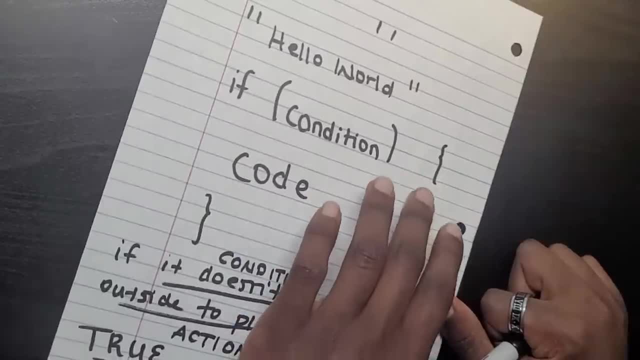 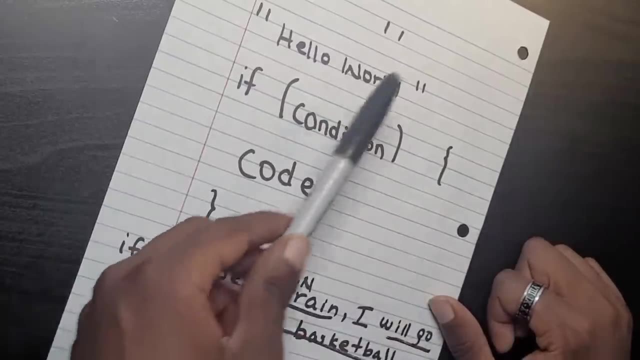 skip it. The whole what, The whole code right here. You can write hundreds of codes in the middle of these brackets, but it's going to what It's going to skip it as long as what? The condition is what? Not satisfied. If it's satisfied, it's going to what, It's going to run it. So I just want you. 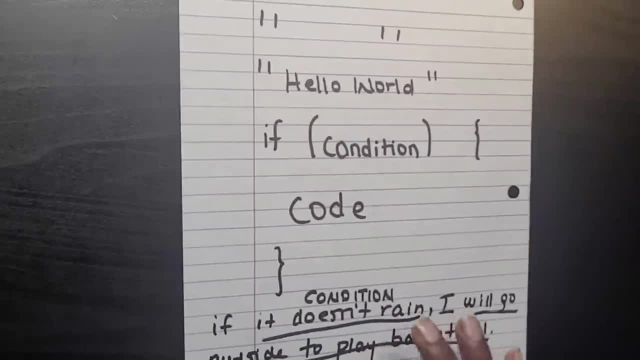 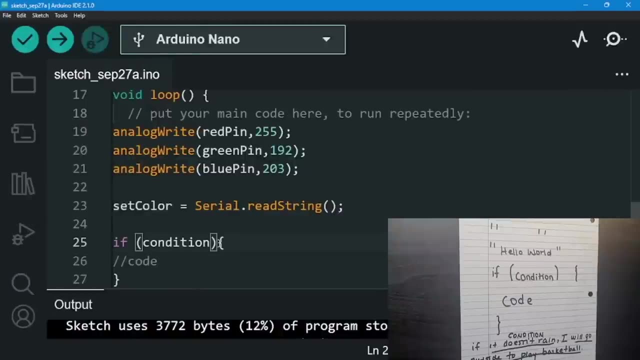 guys to keep that in mind. So what are we going to do with this if loop? right here. What are we going to do right here? So let me go over right here. Okay. The condition here is: what If red? right here. if the set color is what If it's equal to red? okay, If it's equal to red. 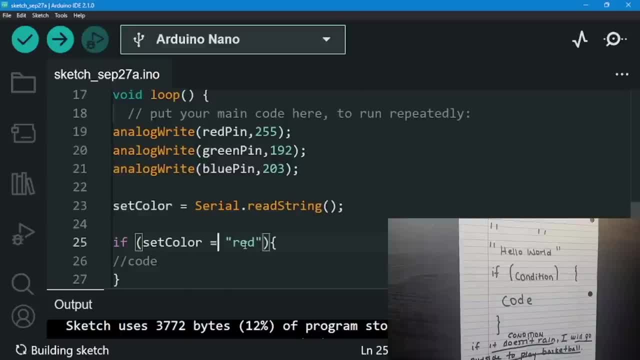 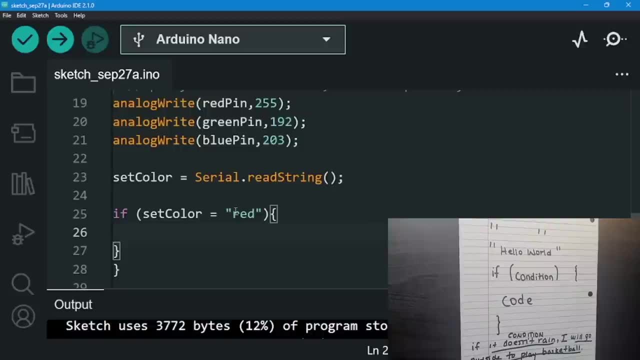 let me see right here, If it's equal to red, what do I want to do? right here, When it's equal to red, what do I want to do? You guys know RGB, so we want to get the most red color. How do we get the most red color? We do what We do, this analog right. So let me copy. 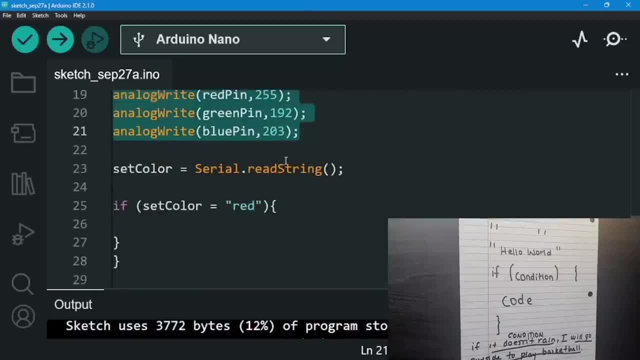 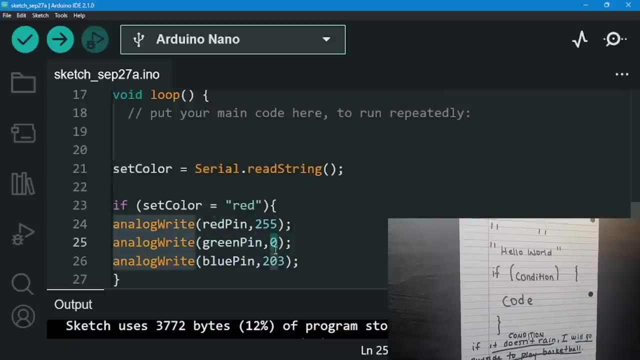 the analog rights and I'm going to adjust the value again. Let me just remove this and let's just print this again And we have again analog what? Red pin, 255.. Analog right green pin for what? We're going to set this to zero. And the blue pin: we're going to set it to zero And the? 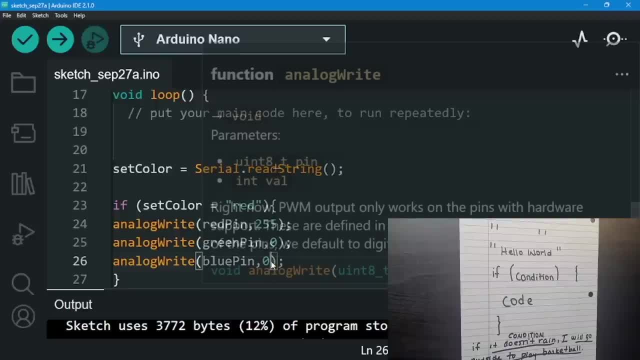 blue pin. we're going to set it to zero Because we only want what, We only want red to be lighting up, Because what we want, the color is what- It's red. So again, we can again use our color picker. 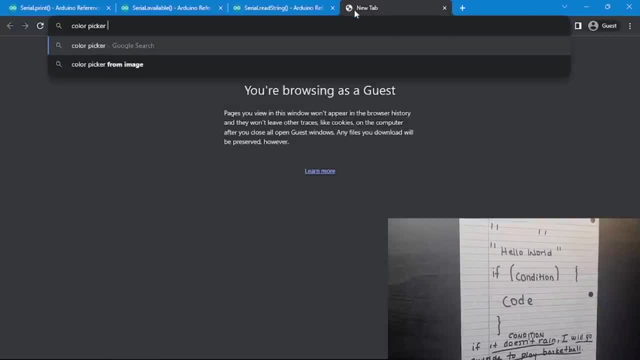 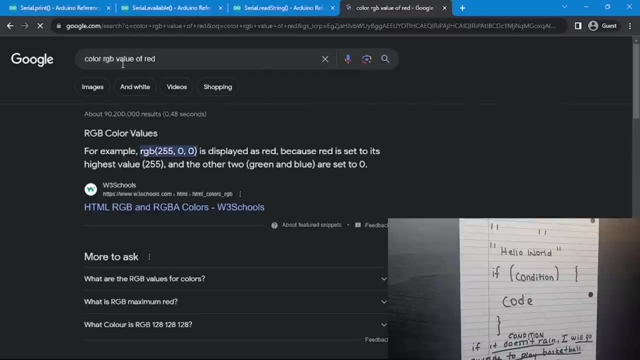 right here. if we want to, We can just go to color picker and say color, sorry, color. RGB value, RGB value of what Value of red? When we do that, the RGB value of red is what? 255, 0, 0.. There we. 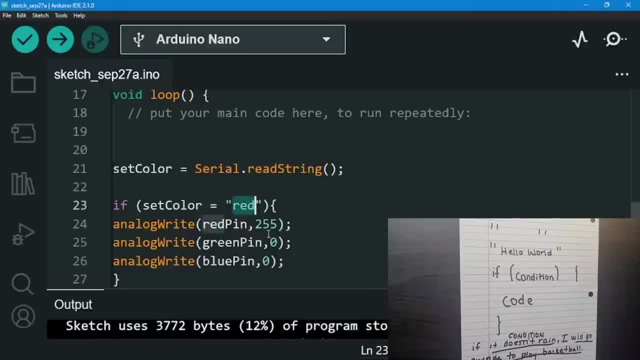 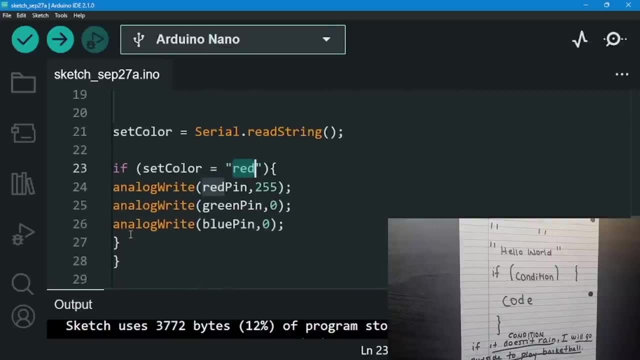 go. So that's what we basically did: 255, 0, 0.. I wanted to do it- and a lot of people don't know what that is, But I wanted to do it. So what if it's not red? So right here, when it's not red. 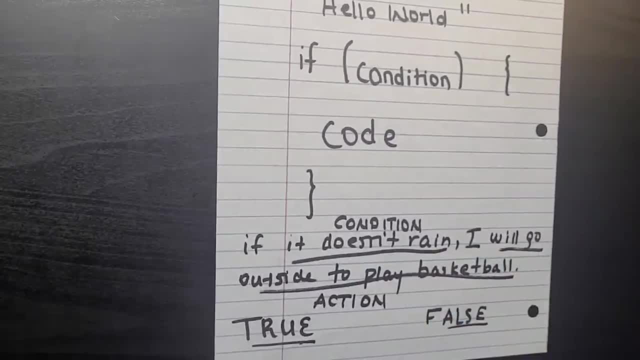 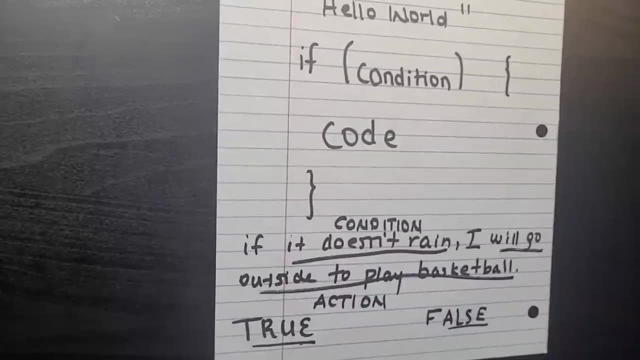 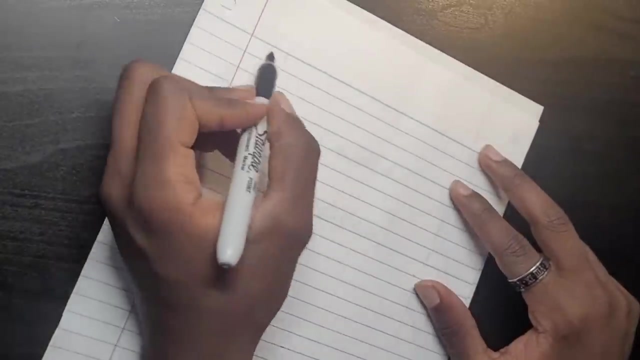 when we want to set another condition. okay, Now let me go back to my paper. Actually, let me add another paper, to be honest, because this paper is not enough. There we go. So how do we set another condition? Okay, We're going to be using something called else. Okay, We're going to. 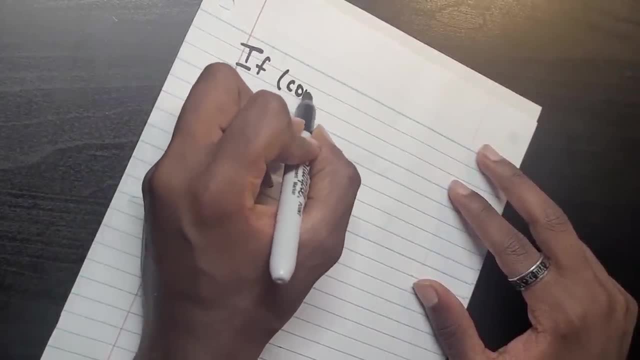 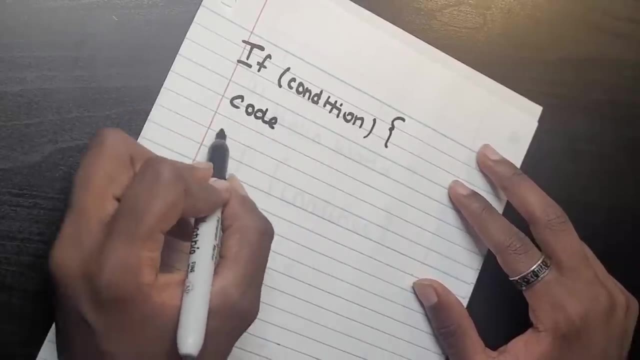 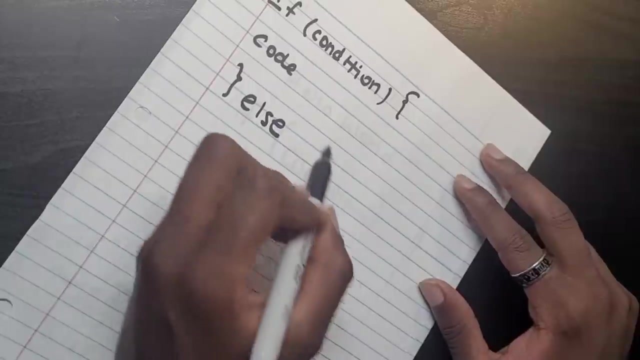 say if, right here. and then we're going to say if, So, if we want to set another condition, right here, we're going to say if, and we have our condition, Okay, And it's going to be running the code. if this is true, Okay. Okay, Then we have something called else. Okay, Else, Else. 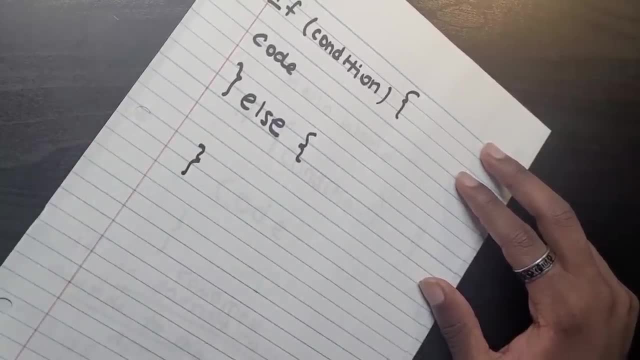 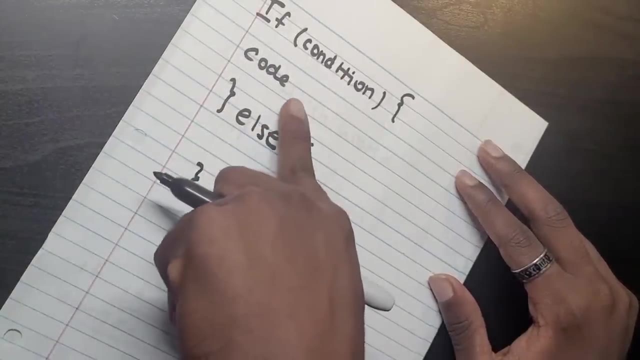 as in what It's the second option, Else is what It's more of what The second option. So if this condition, for example, is satisfied, what is going to happen? It's going to run the code, as I said. But what if this condition is not satisfied? If this condition is not satisfied, 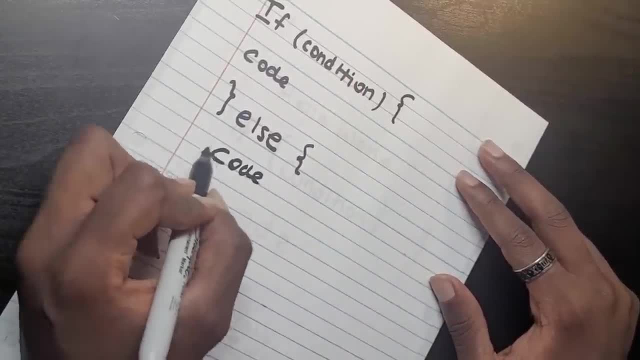 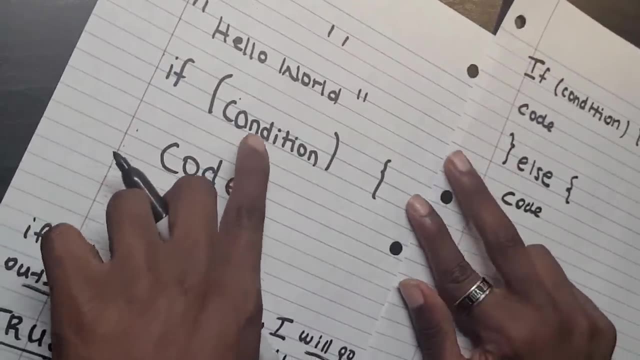 I want it to run, let's say, a specific code right here. I want it to run a specific code right here. Okay, Instead of just, you know, skipping it as traditionally, what does it do? It had a condition and a code. If it again this condition is not satisfied, what did it do? It just skipped. 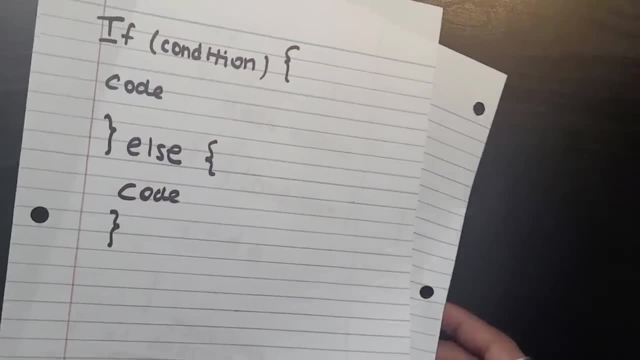 it. But let's say I want to you know, if in this case this condition is not satisfied, Okay, In this case this condition is not satisfied. If in this case it's not satisfied, what I want to do. 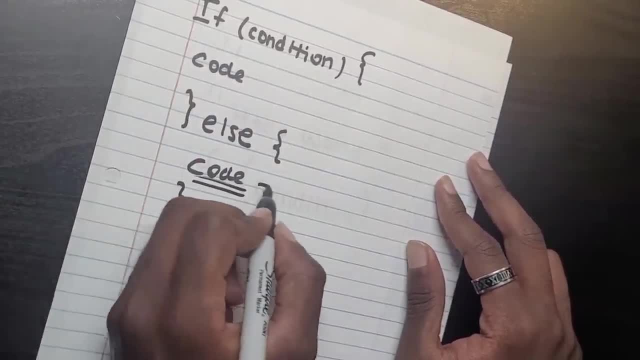 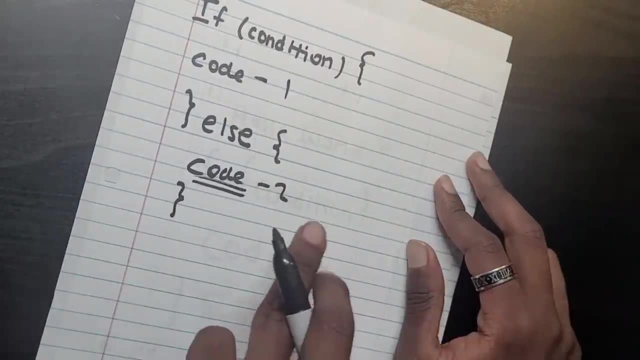 is write another type of code. right here. We have code number two right here and code number one. I want it to write code number one if this condition is satisfied, But if it's not, I want it to run another code. Okay, Instead of just skipping it, I want it to write another code. That's why. 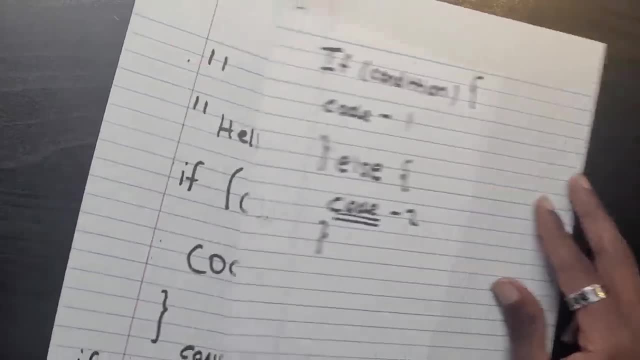 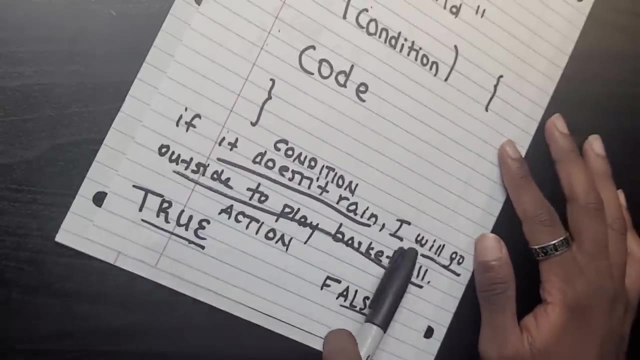 we're going to be using something called else. So what I want you to think of them is like this: Okay, We have this again sentence right here, which was what? If it doesn't rain, I will go outside to play basketball. Okay, But something else can happen to other than raining. Let's say: 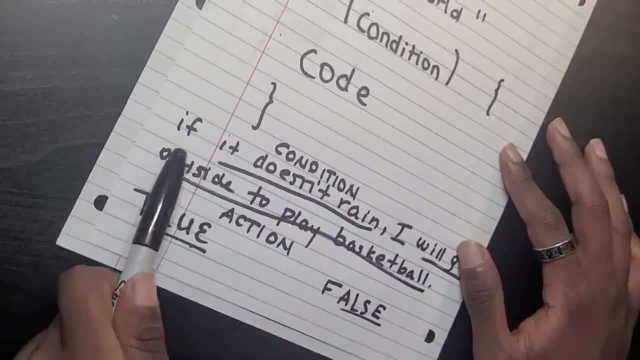 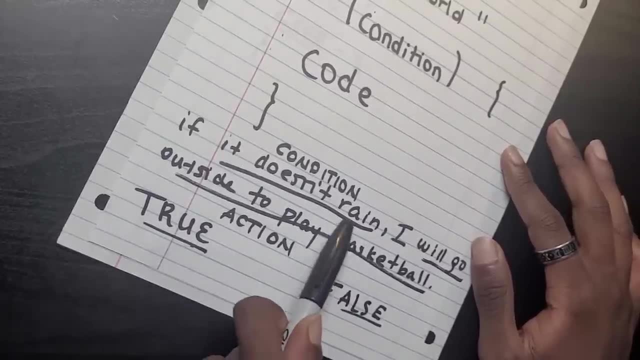 it gets too hot. I'm talking really, really hot. So if it gets too hot, what happens? If it gets too hot, what happens? I will not go outside and what Play basketball. So, instead of just about, we're only talking about raining here, which again has a what? A wider context, Because 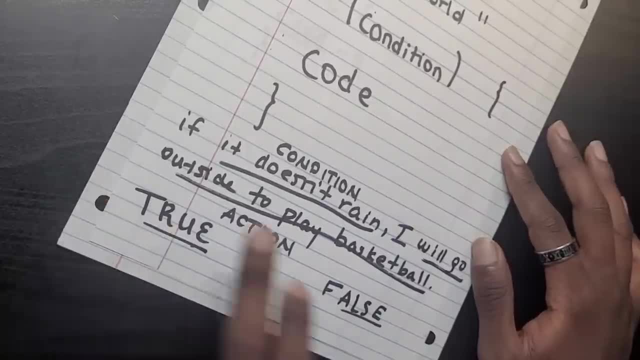 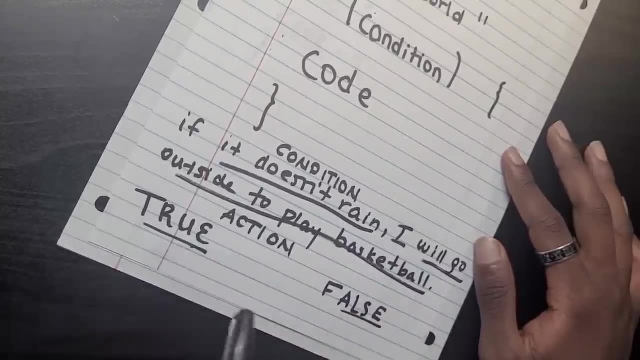 let's say it's, there's a tornado, let's say outside, If there's a tornado or a hurricane outside, what I will not go outside and play basketball. Obviously I will not go outside and what Play basketball. So I just want you to keep that in mind, So when you're working with else, 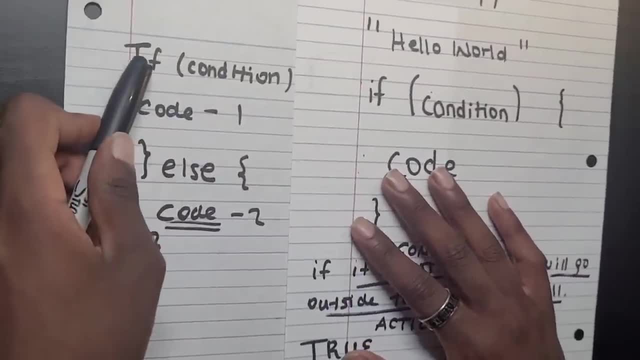 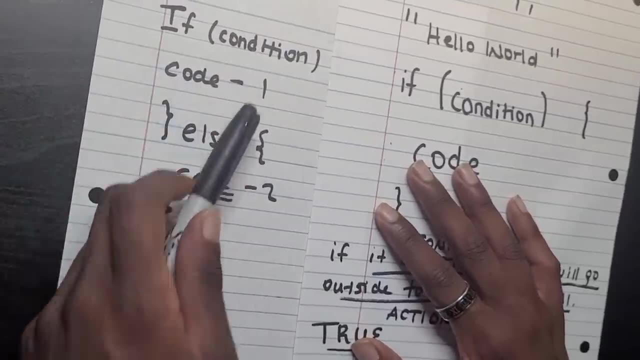 what are you doing? We're just adding another condition. We're just adding another condition. We're just adding another condition. Basically, what we're saying is basically: oh, if this, what? If this code is not run, its condition is. 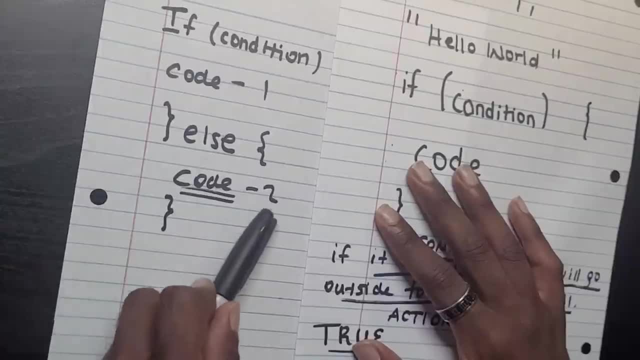 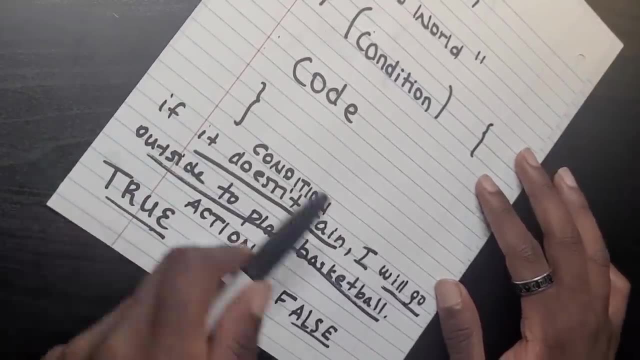 not satisfied, I'm going to give you another option, which is going to be writing down the second code. Okay, So I just want you to think of it as that. So, if this, what? If this condition is not satisfied, I want it to do something else. Okay, Instead of just not playing basketball. 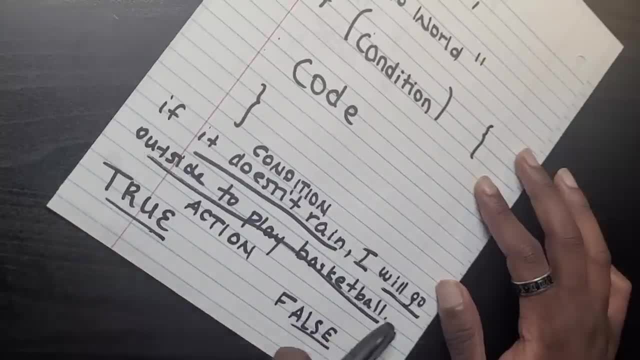 I want it to do something else. One of it would be what? Playing? maybe board games, Okay. So if let's say, if it rains, okay, if it rains in this case, what is it going to give me? 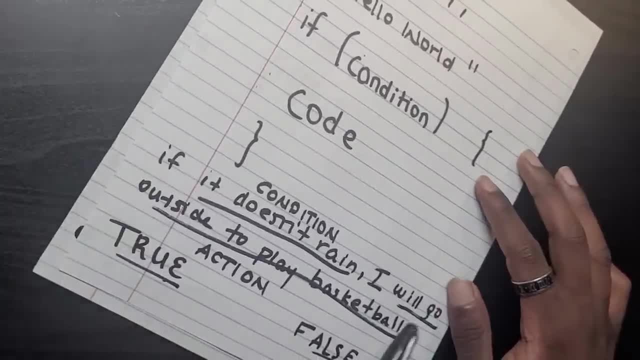 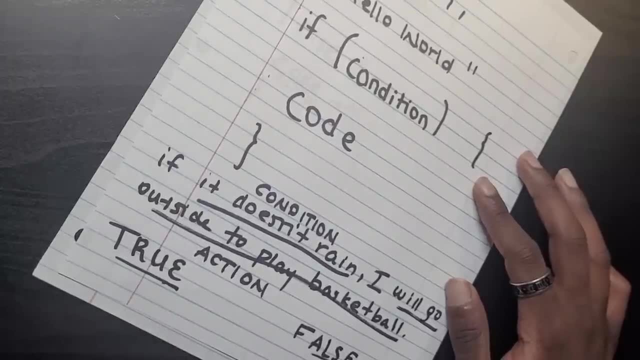 Our condition is going to be what False. If it rains, instead of just not playing basketball, what else am I going to do? What else am I going to do is what I'm also going to be, let's say, playing board games inside the house. Okay, With my friends, Let's just say that, Okay. 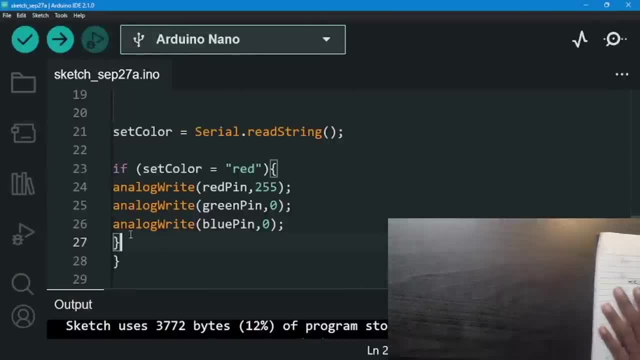 So, with that in mind, okay, you can say, is what else? Okay, Else. And what I wanted to do is I wanted to tell our user: right, here, I wanted to print out and tell our user: right, Let me just go to serial dot, print and tell it. 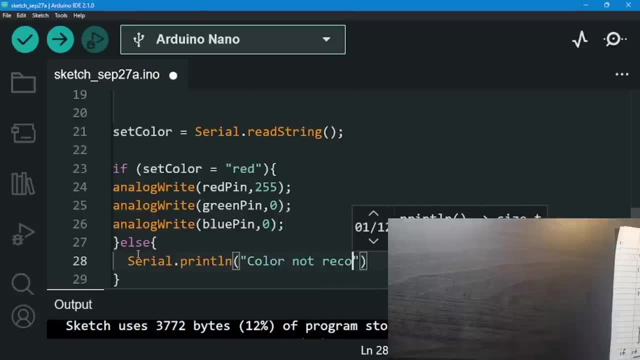 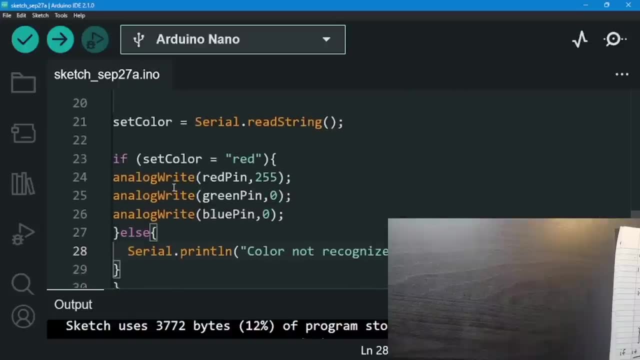 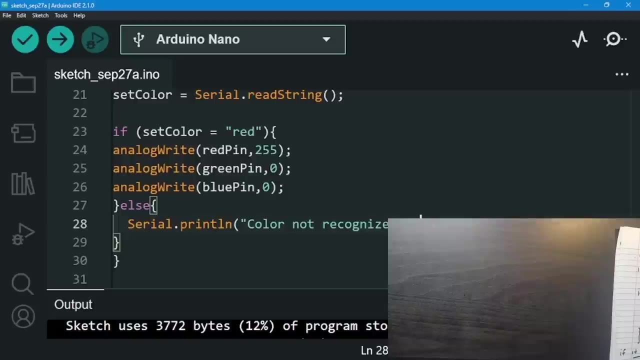 Hey, color not recognized. I wanted to tell it that we do not recognize what color it said right here. Okay, I just wanted to tell it: oh, I don't recognize the color that you're saying right here. Okay, All right, That's what I want to do, Okay. So one final thing that we need to learn about. 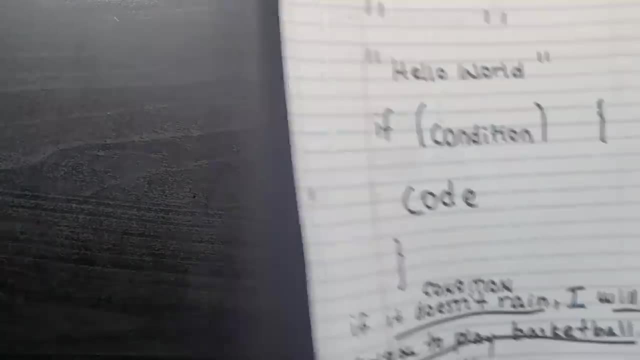 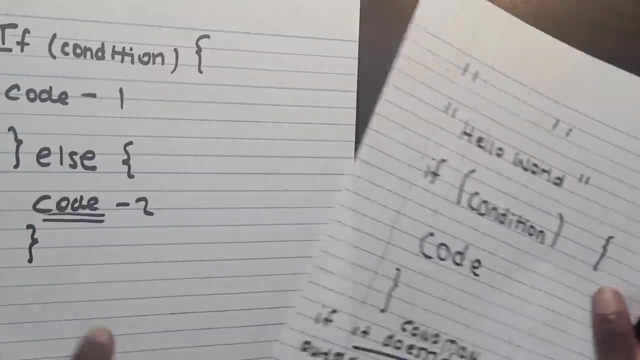 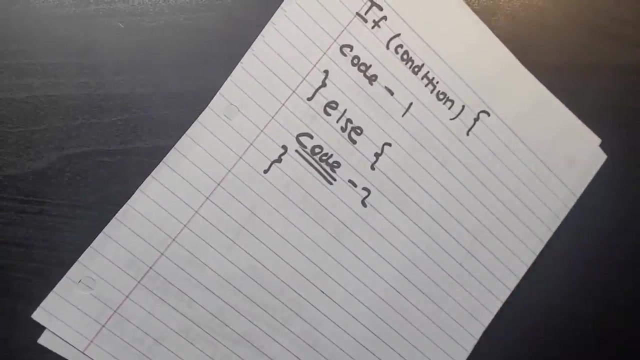 if and else is to be exactly fully done is something called. So we learned about if right here in the street cap. we learned about, And then we learned about if and else, combining them together, And then we're going to learn about something called if. right here, let me start. It's going to start like if it's going. 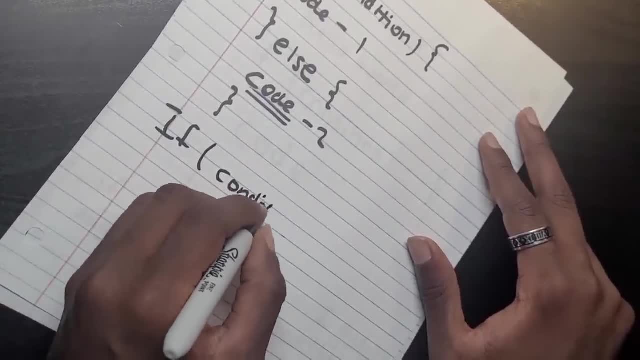 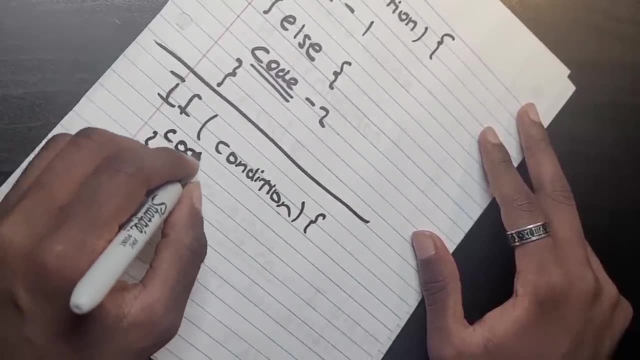 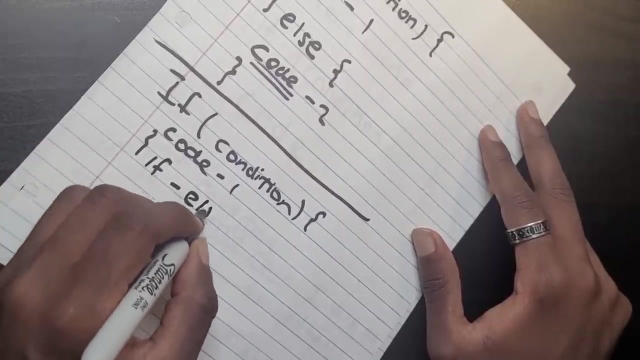 to add up to it. And there's our condition. Let me just give this and separate this condition. Obviously, we have our code in the middle of the brackets. It's going to be code one. Then we have something called. if else, All right. 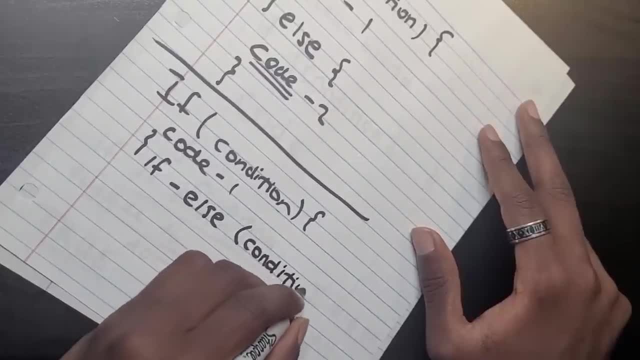 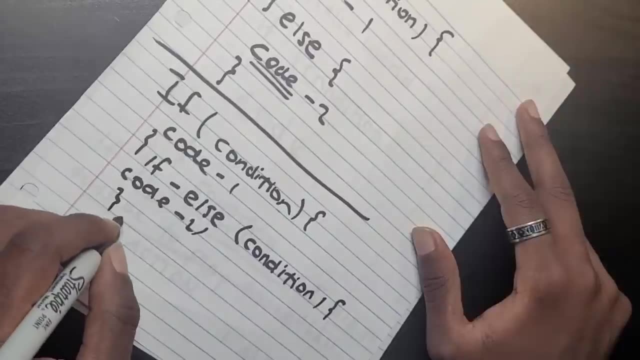 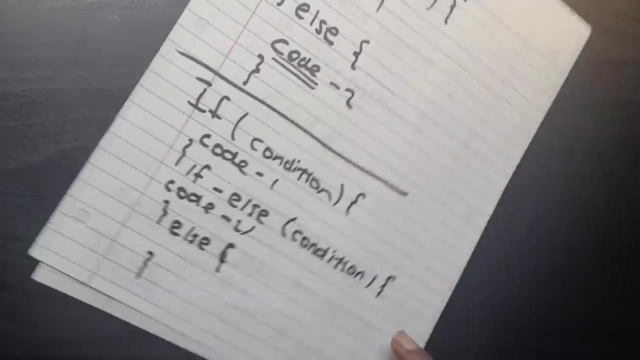 And we have a condition again, we can write down another condition. Okay, We're going to be using code two again, right here. And we can even set it up with what with else? right here, Again, right here, else as well. It's the final straw, Okay, So here we go. So what does this mean? So, this means: 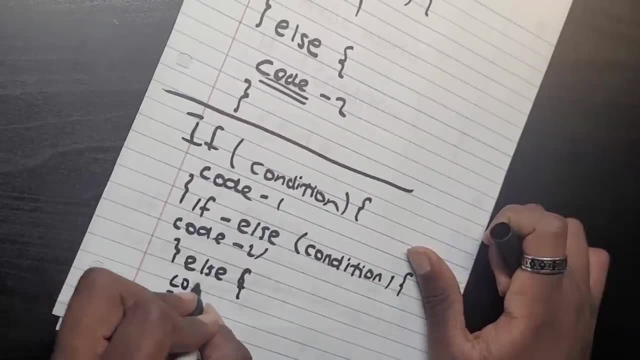 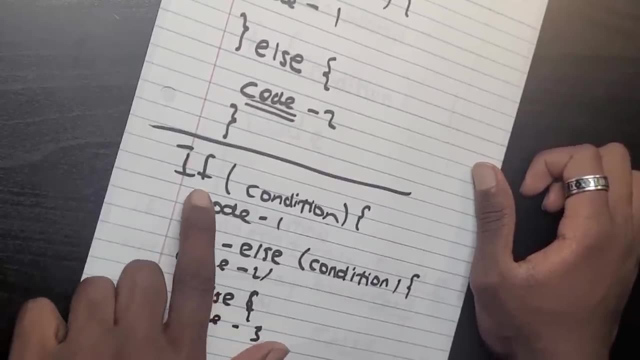 is: oh, we have our code three right here, When you see else, we have our code three, We have a third code. There you go. Okay, So what does this mean? So this means is: look if there is a condition, what's going to? 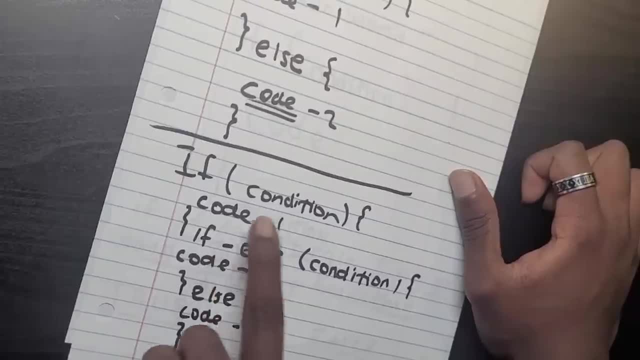 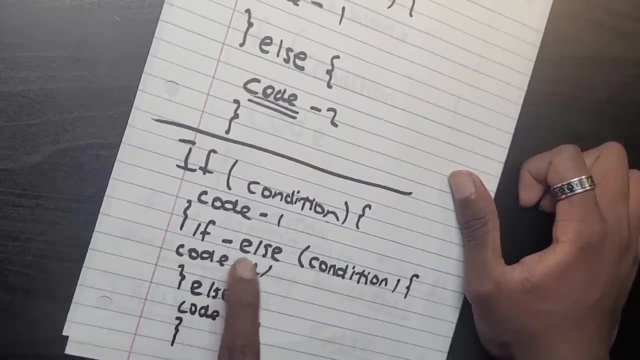 happen, It's going to be running the first code. If this condition is not satisfied, it's going to go to the second one. We're going to give it another condition. Okay, So we're going to give it another condition And it's going to be what? Running code two And what The third one is going. 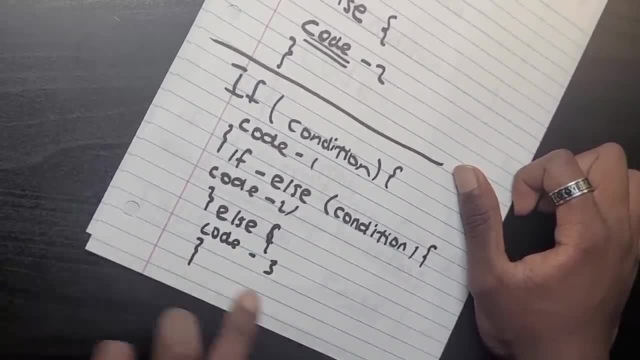 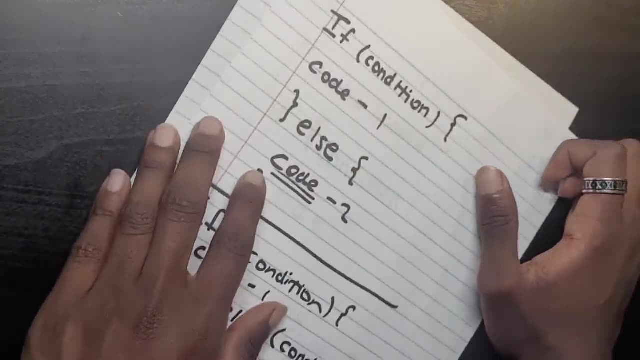 to be what It's going to be: running the final straw It's basically what. The final straw It's like the final, you know, like the final thing that you do. when you have anything else, you don't do, right, You don't do anything. When you don't have anything else to do, you don't do anything. 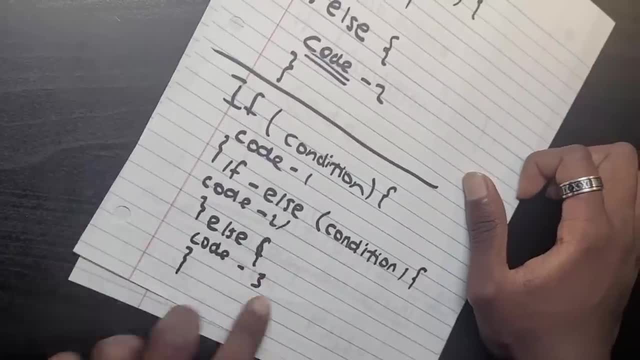 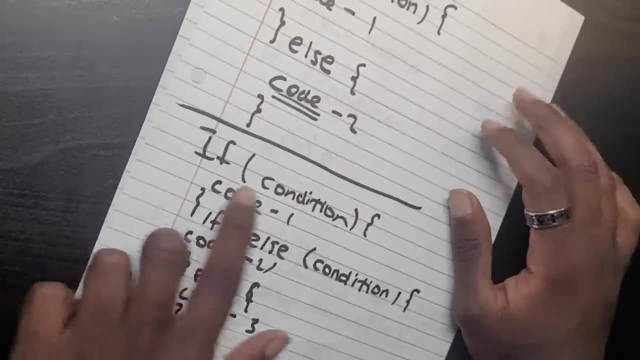 When you don't have anything else to do. it's like the final straw- Okay, It's going to be running what Our final straw right here. So I want you to keep that in mind. So there's if again condition with the code one, and there's if else condition and our code two. and then what else? 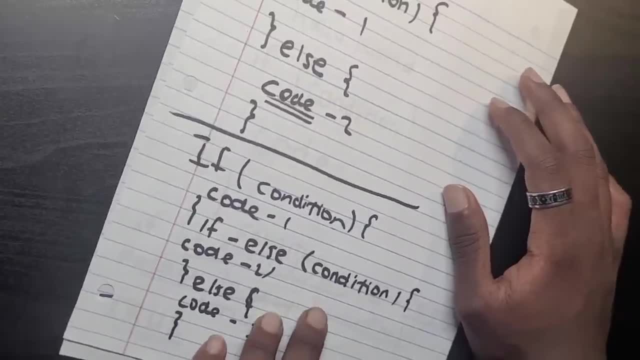 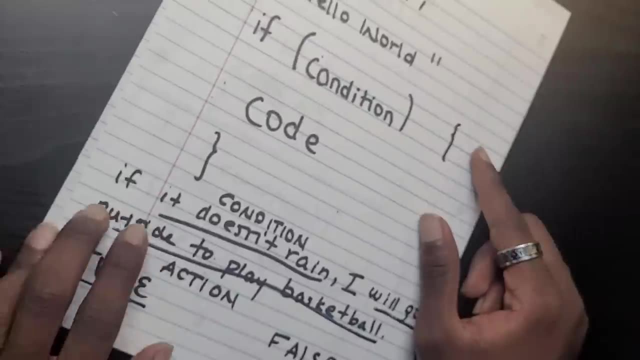 and then our code, the third code. So I want you to keep that in mind, Okay. So right here, let me just bring my again our simple example right here. I think it's going to make it way easier. So what's going to happen? So what's going to happen? So what's going to happen. 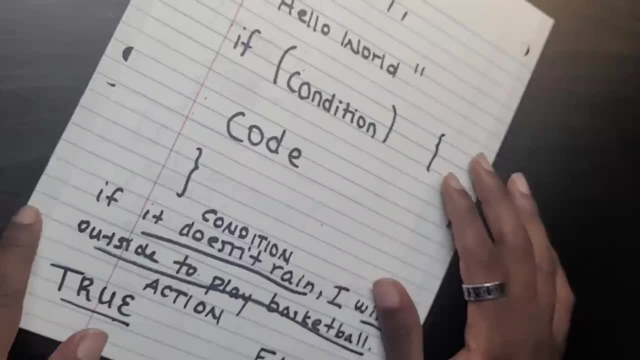 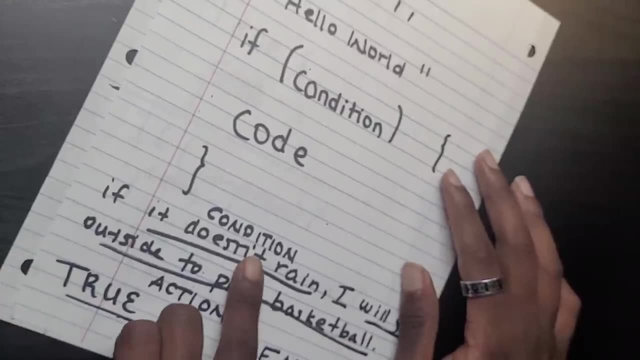 What does an if else fit right here? So it's basically thinking of it. as I said again, if it doesn't rain, I will go outside to play basketball, All right. So in this case, let's say it rains, Okay, When this code is not satisfied, it's going to jump this one, And what's going to? 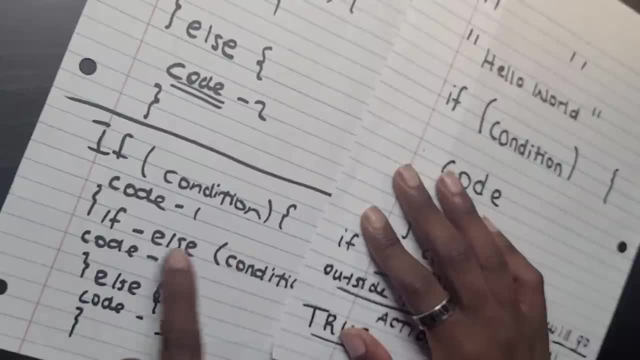 happen is, if else, it's going to go to the, if else, right here, the second option. it's going to be the second option. It's going to go to our second option and say, okay, it's raining, What else can? 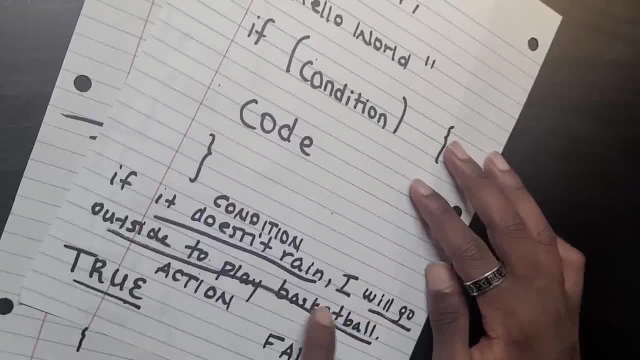 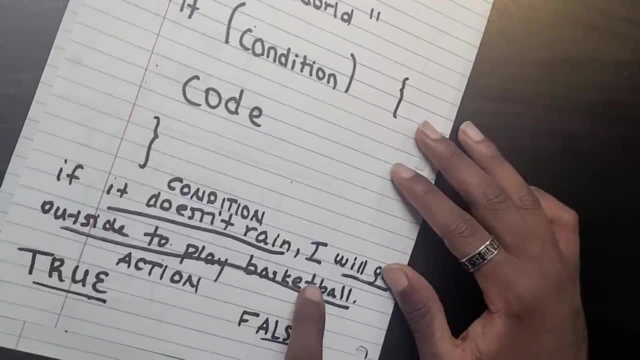 I do. What else can I do? Okay, I'm not going outside What? I will not go outside to play basketball, That is true, I will not go outside to play basketball, but what else can I do? I can be on my phone. Let's say: okay, let's say what I can be on my phone. I just want you to think of. 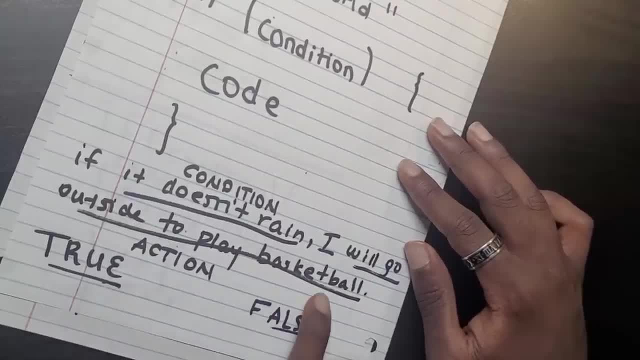 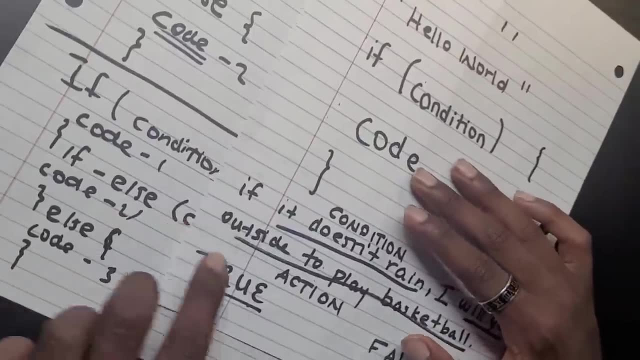 it as well. I will be inside of my house and be on my phone. Okay, All right. Then let's say again: there's another condition where this one cannot be true. Basically, let's say there's no light and my battery's dead. Okay, Let's say my phone battery's dead. In this case, let's say my phone. 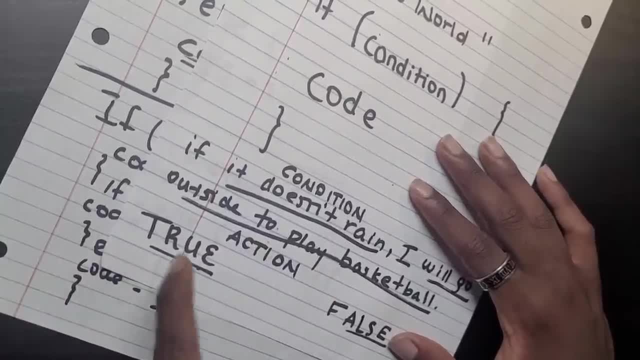 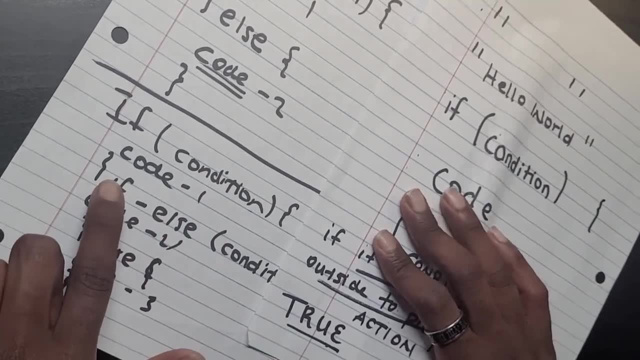 battery's dead. As a final straw, what do I do? I play board games because I have nothing else to do. That's what I want you to think of. Okay, So, when this condition is not satisfied, there's what. There's what? When this condition is not satisfied, we have another condition that we're. 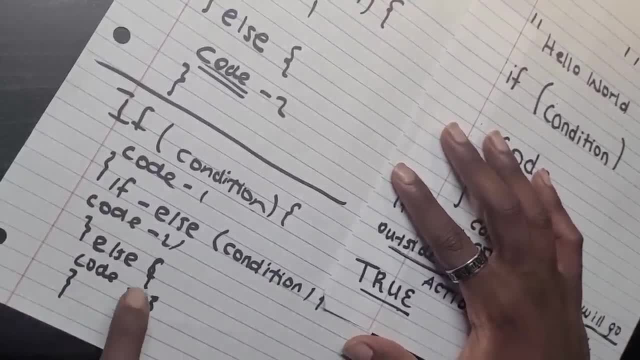 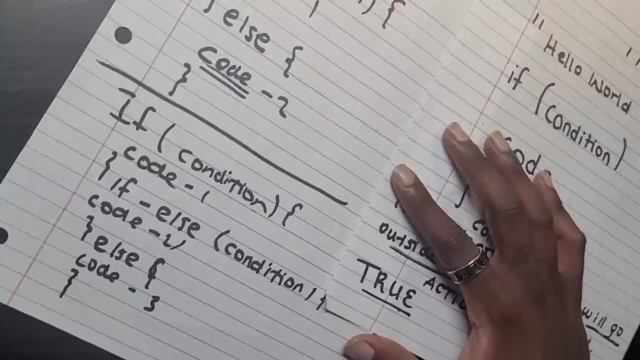 going to do. But when that condition is again not satisfied, we have a final straw again to do what To do? our last thing, Okay. So let's say then we don't have board games. Well, let's say this is: 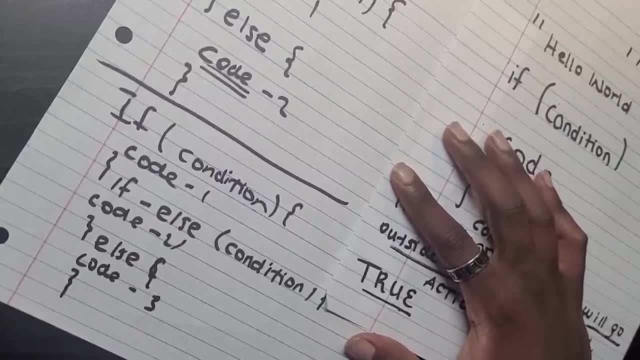 going to be another. if else, Okay, We don't have a board game. What are we going to do? Okay, What we're going to do is maybe we'll sleep, because what We don't have- any board game We don't have. 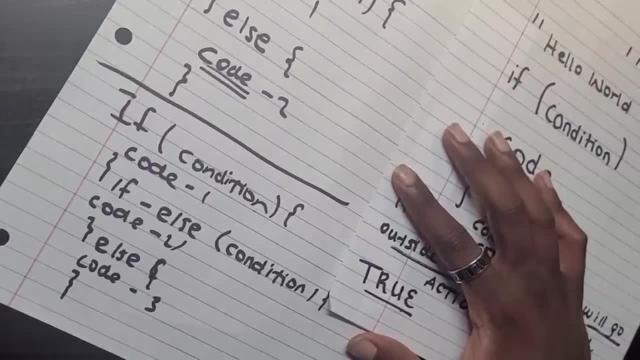 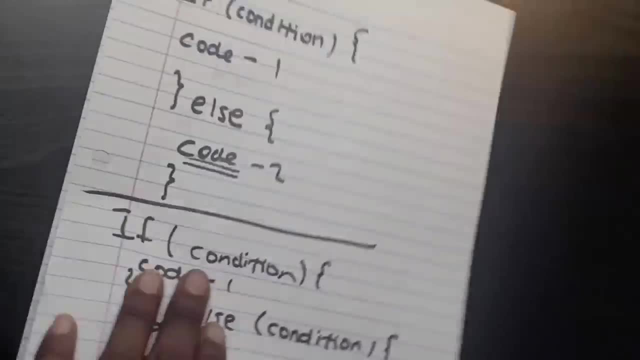 anything to do. Basically, we don't have anything. We're just going to go to sleep, Okay. We're just going to take a nap, All right. So that's why I want you to think of them, Okay. So one thing you always need to keep in mind when working with 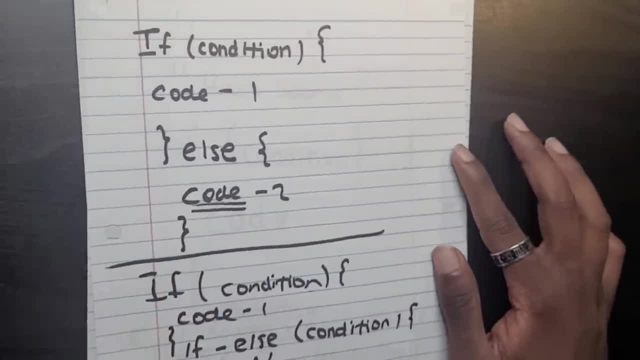 these is what It goes from up to top. The one thing you want to keep in mind is what It goes from up to top. So again, from up to bottom, up to bottom. So it's going to be reading the F right. 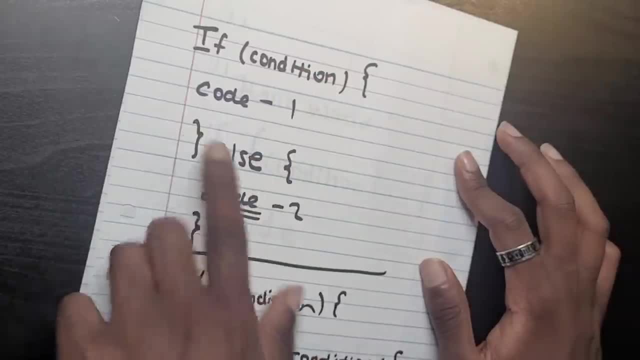 here. So let's say it reads this one And this is true. If this is true, what's going to happen? It's not going to read the else one. Okay, It's not going to read it. It's not going to read it. 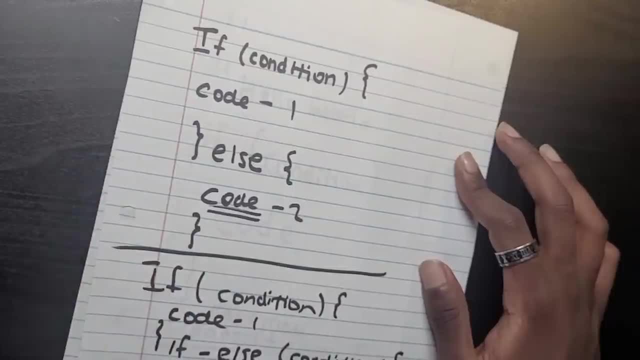 It's going to skip it. It's going to what It's going to skip it. I don't know what thing you're writing in. It's going to what. It's going to skip it. Okay, Keep that in mind. When it comes to this one, too, what's going to happen is it's going to read the. 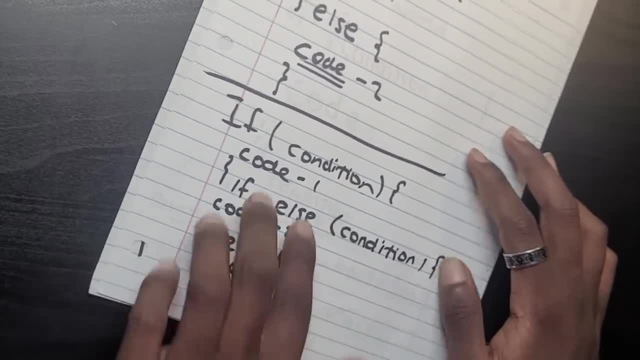 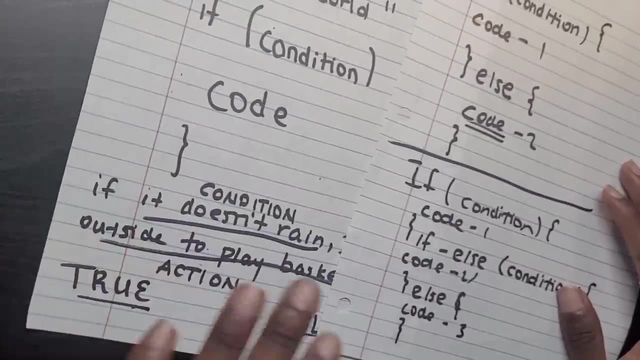 first condition. If the first condition is satisfied, what are we going to do? Let's see in this condition, for example, if what? It doesn't rain, What do I do? I just go outside and play basketball. I'm not going to be on my phone, I'm not going to be using board games or anything. 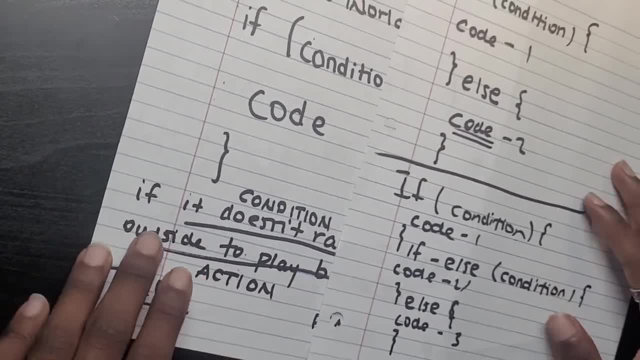 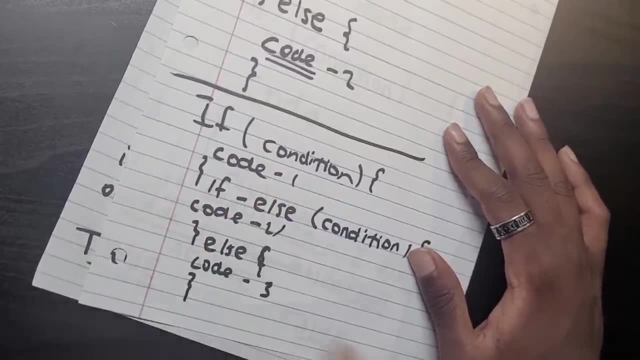 I'm going to be what I'm going to be what Playing outside. I'm going to be outside and what Playing basketball. So I want you to keep that in mind. So, when this condition is what Set to true, It's not even going to read the last options, Okay, So 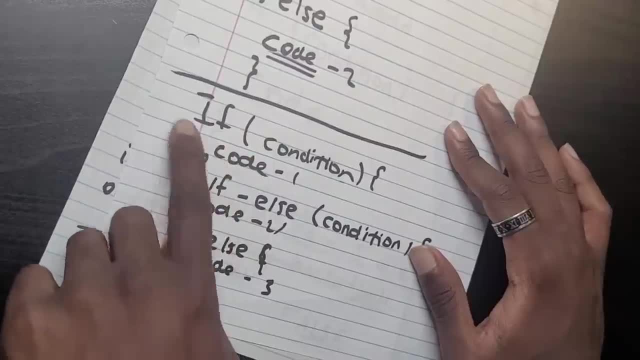 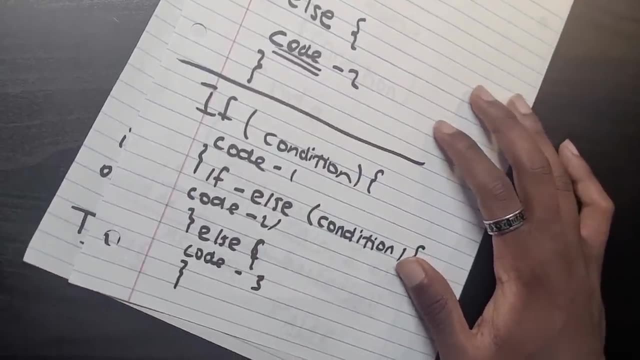 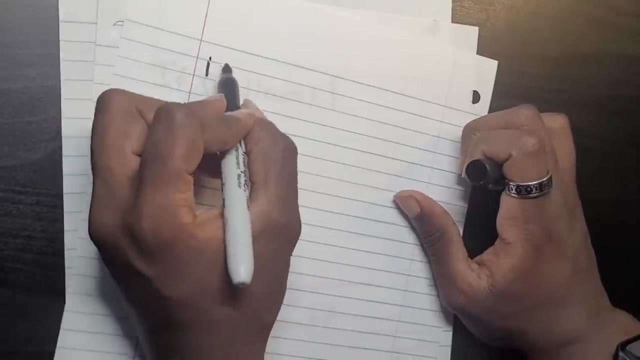 it's going to pick from these options, And the first option is obviously this: If it reads this- and this is true- it's going to skip all of this, Okay. So one final thing that you need to keep in mind is you can write down if- Let me just bring this here: You can write down if, And then. 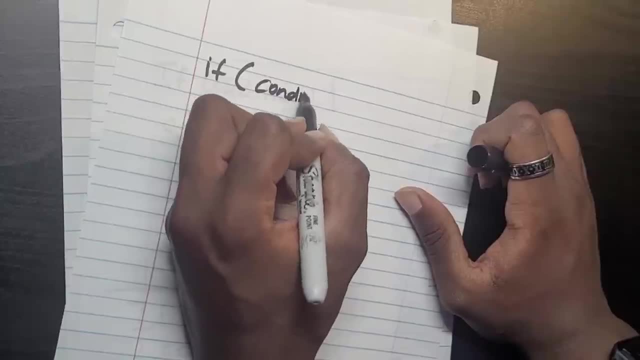 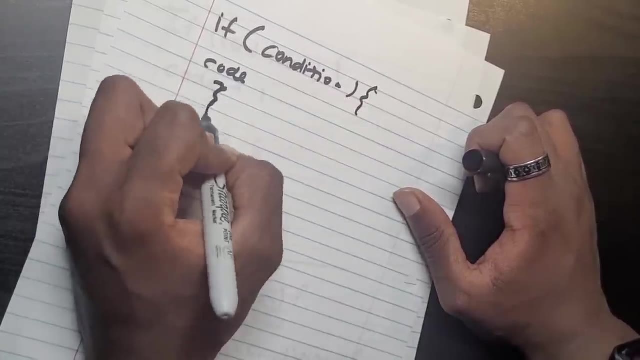 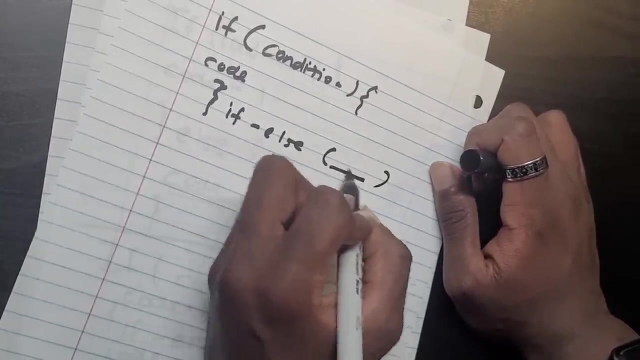 you can write down what, Write condition, Again the condition, And then our code is going to be written down. We obviously what, We obviously write it down Right here, Then we have. if else, Okay, Then again it's going to have its own condition here. 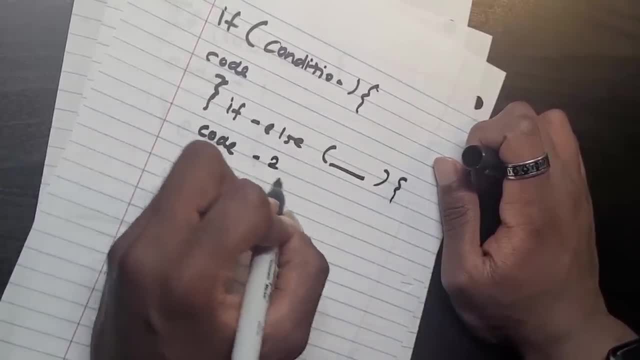 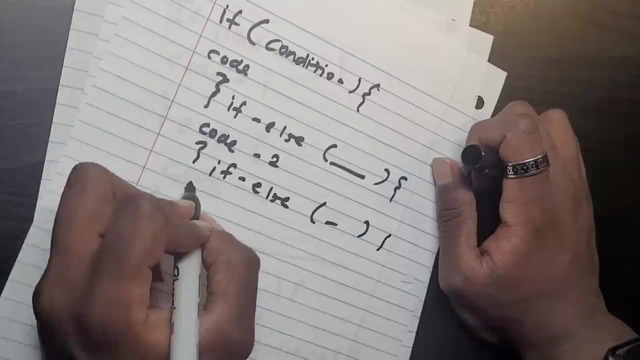 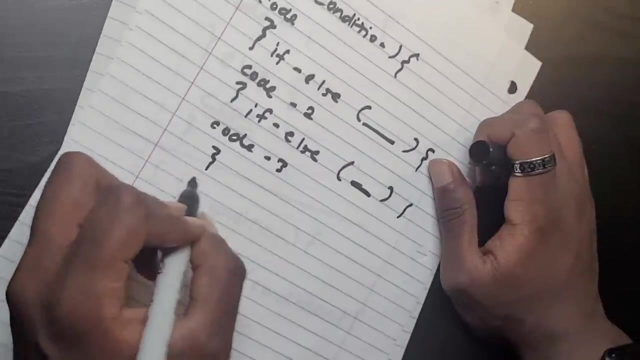 And it's going to have its own code. It's going to be code two. Then we can also add another. if else The same thing, It's going to run another code with another condition. It has another different condition right here: Code three. If else, You can keep adding it. to what? 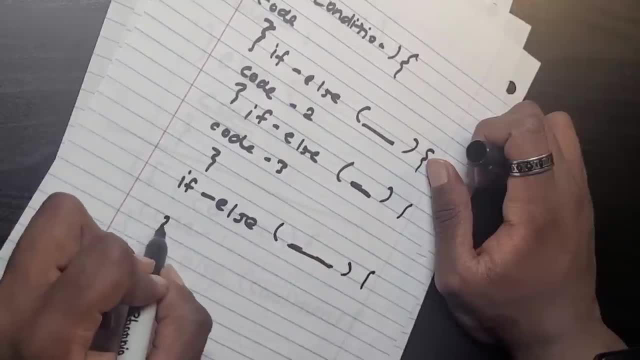 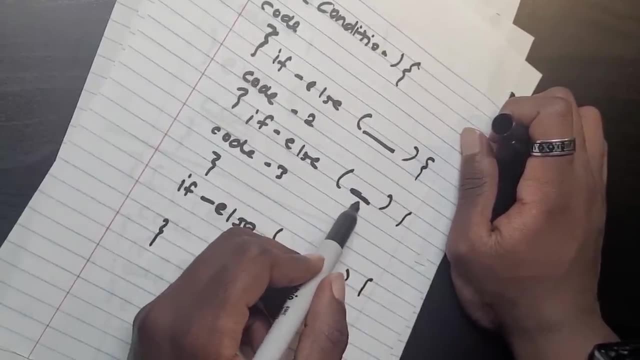 To infinity. Okay, You can keep adding it to infinity. You can keep adding it to infinity. Right here, It's like adding: let's say: okay, I don't have, you know, my phone's not here with me- Okay, I'm going to be reading a book. You know what, Instead of reading a book, I'm going to be. 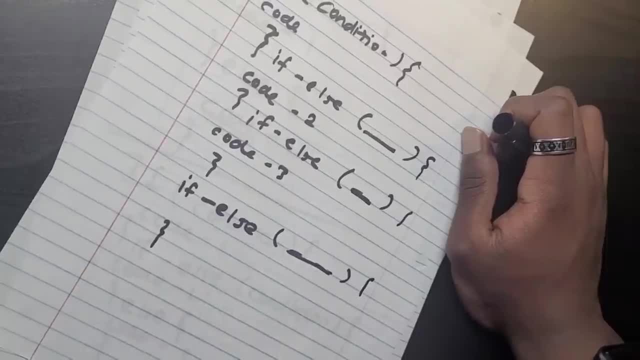 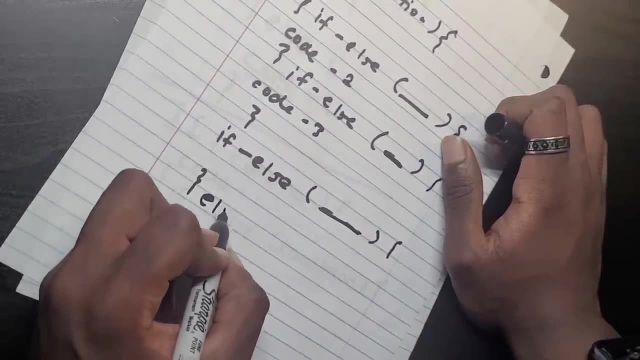 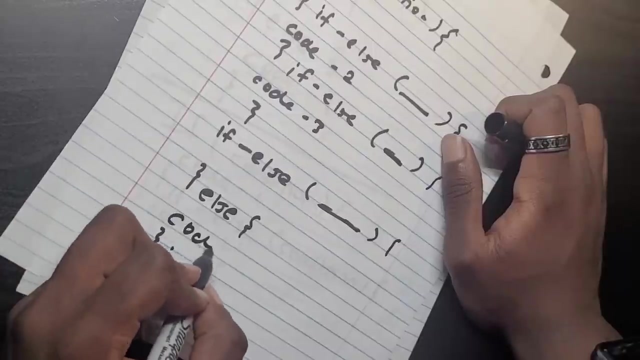 cooking dinner or something, So what. There's like infinite possibilities. Okay, So you can keep writing down- if else, What Infinitely? And then at the end, what you do is always finish it with the last option- It's going to be an else right here- And you finish it with a code. So 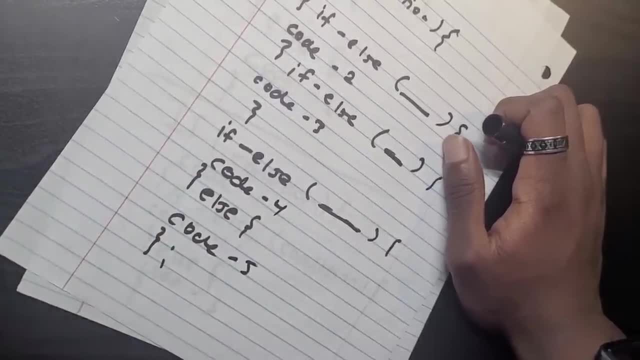 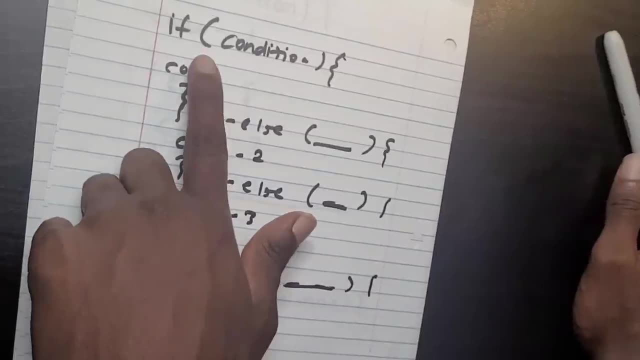 this is what Our code Four. It's going to be our code five. So one thing I want to again, as I said, is what Always one of it is going to get picked. So what's going to happen again When this is picked? 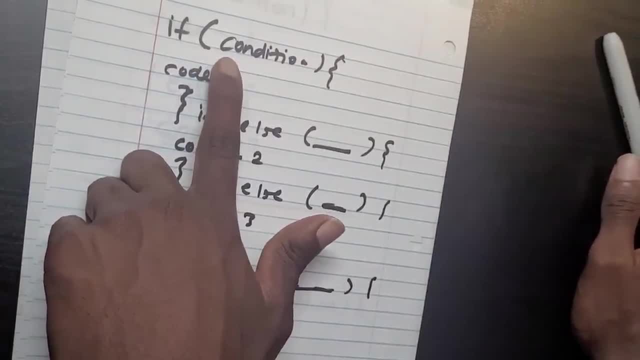 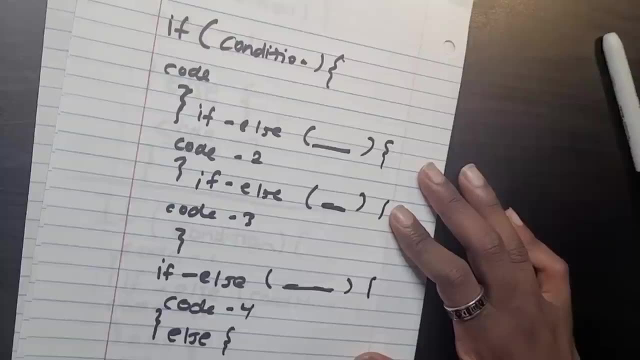 if the first condition is picked. what's going to happen? If the first condition is picked, what What's going to happen is basically what It's not even going to read all these. If this is true, it's not going to read any of these from else All of it, till else Everything. It's not. 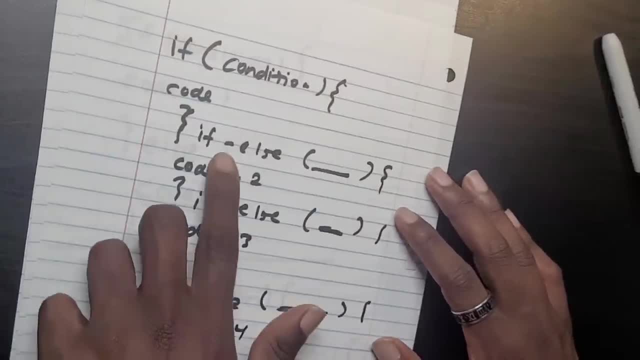 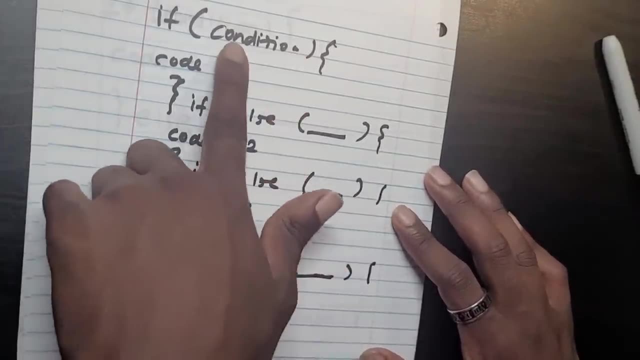 going to read anything. It's not going to read all of it, All right. What if the second condition is true? The second condition is true. What's going to happen? Okay, First reads the first condition and this one is false. and second condition, let's say it reads it and 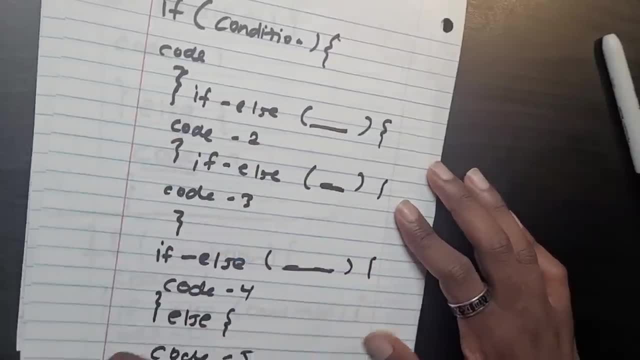 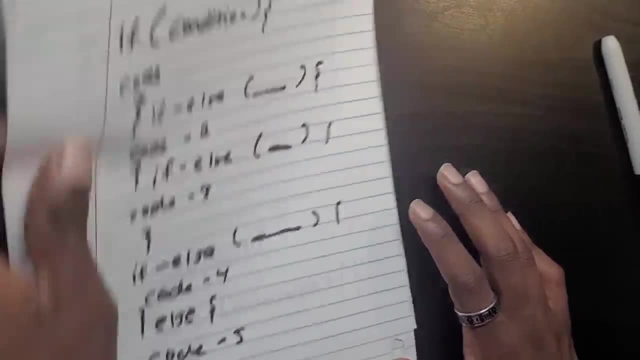 it's true in this case. what's going to happen? anything beneath it is not going to be read. it's going to be what it's going to be skipped. anything beneath it's going to what it's going to be skipped. okay, it's going to be. keep going on like that. so i just want you to keep that in mind. we're working. 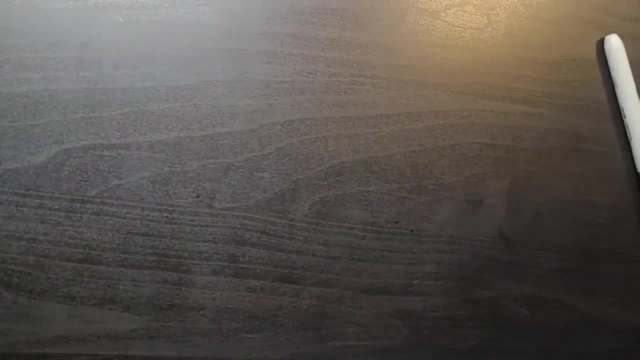 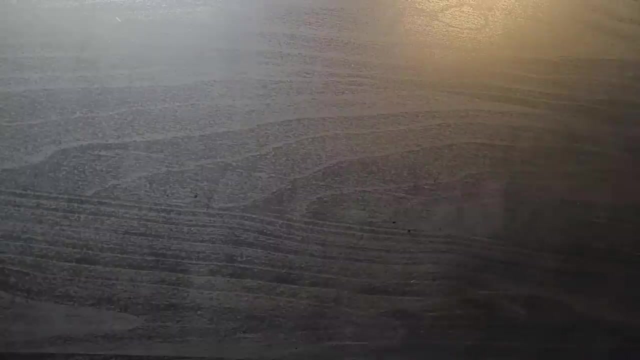 with um if conditions. so i think it has been a very longer section of the course because we're learning about new uh, uh, programming again, functionalities and all. so it's going to be a bit uh, it is a bit longer one. so what i'm going to do is i'm going to stop this right now, right here. 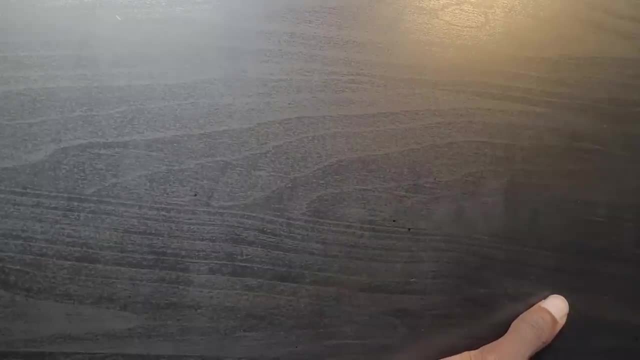 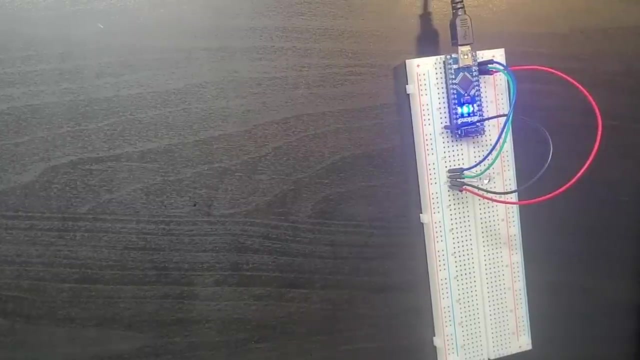 and then we're going to see- uh, we're going to take a break and then see you in the next section. okay, so in the previous section we discussed about if loops and, uh, now we're actually gonna utilize them in our project, so we're going to fully utilize them. okay, so let me go to my screen. 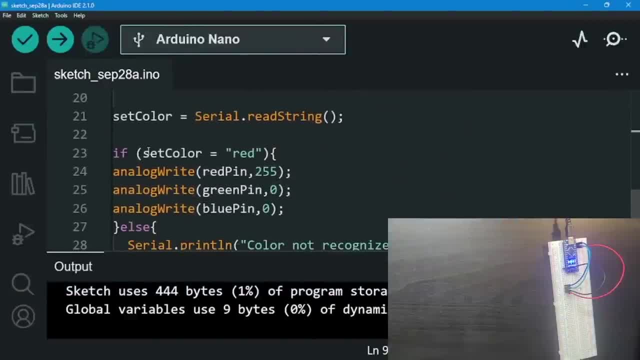 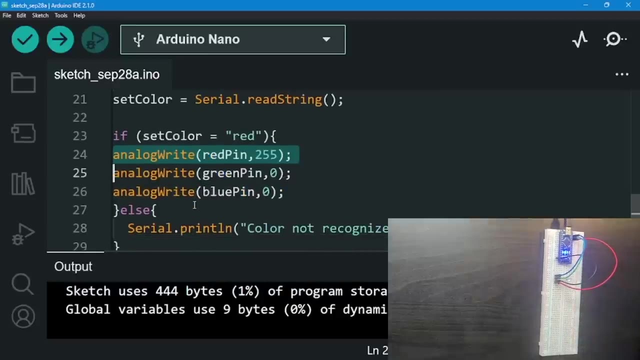 right here. and what does this mean? this is what if the set color is red? what happens? the analog write command. so here, the analog write command. it's going to set the red bit 255. obviously other ones are going to be set to zero, basically giving us what? the color red. so let's see what happens when i just do that. 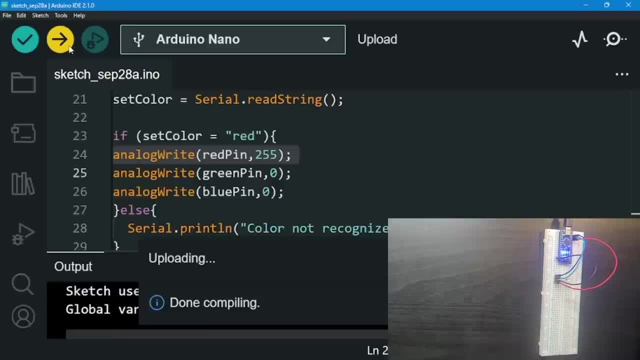 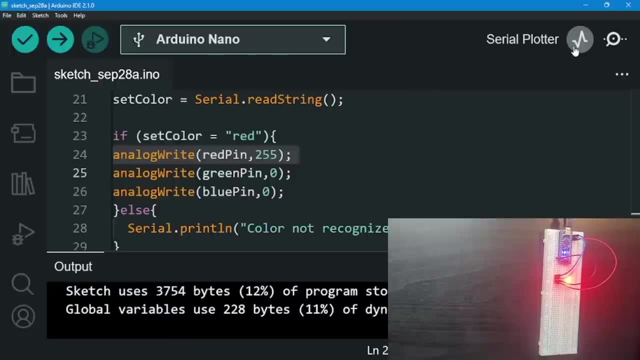 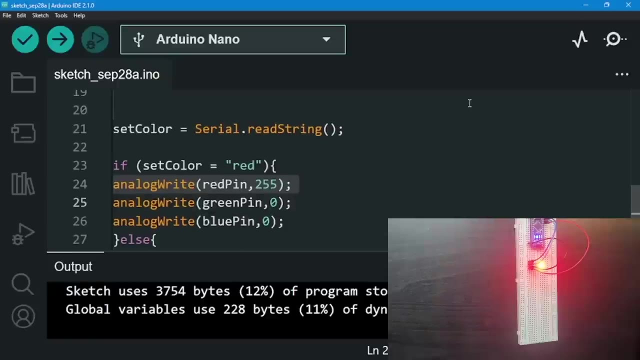 so let me just upload it right now. it's uploading, okay, and there's a problem right here. can you see? i did not write down anything on the what on the arduino. i'm not writing down anything, but what happened here? what happened was it turned down to red, which is a bad thing, because i'm supposed to what i'm supposed to go to my 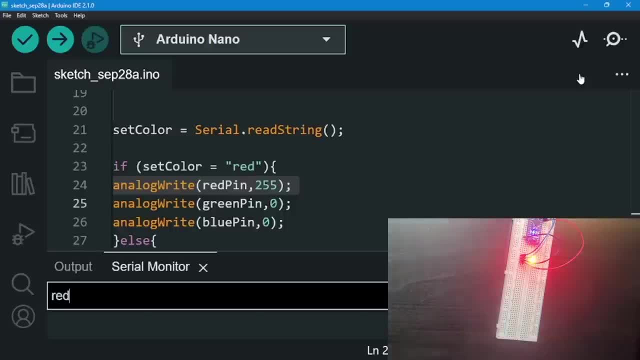 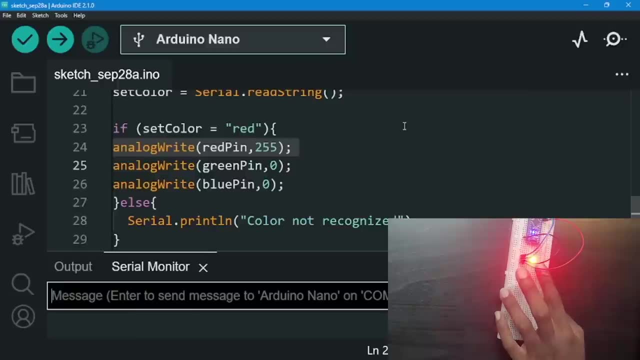 serial monitor right here, and then i'm supposed to type red, and then when i enter it, when i send it to the arduino, then it should have been turning to red, not when i again just did not do anything right here, okay, so i did nothing and what happened was, let me tell you, 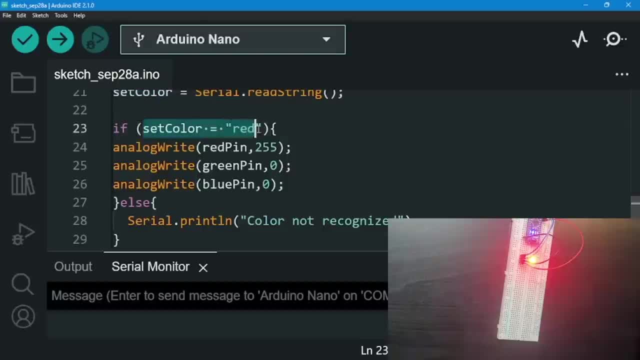 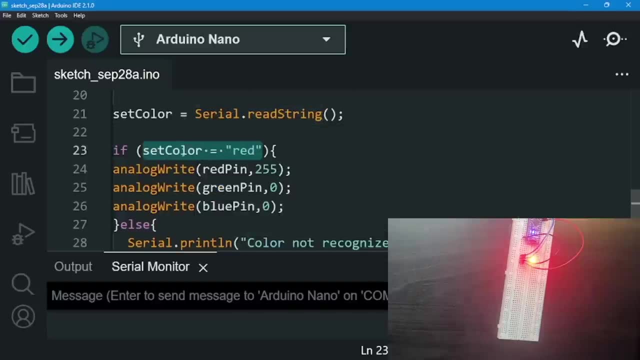 guys, what happened was i said: the color is equals to what to red. right here i said: the color is equals to what serial dot read string. all right. then afterwards, what did i say? if set color is equal to red, i set it to what i set it to read to red. so how do we compare things? so how do we you? 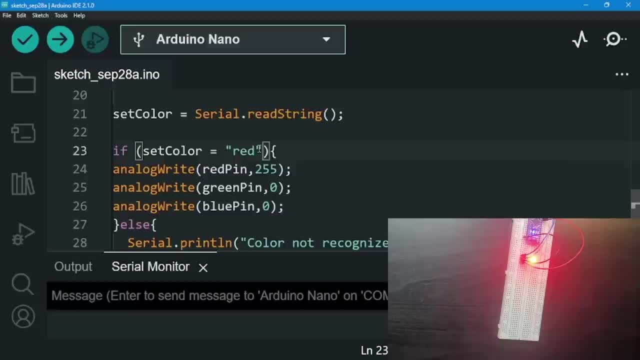 know, know the difference between setting up stuff. you know just as in like this. let me just bring this here, to bring a paper, and i think i'm going to use a math analogy again because to make things way, way simpler for you guys. so i'm gonna bring the paper here. 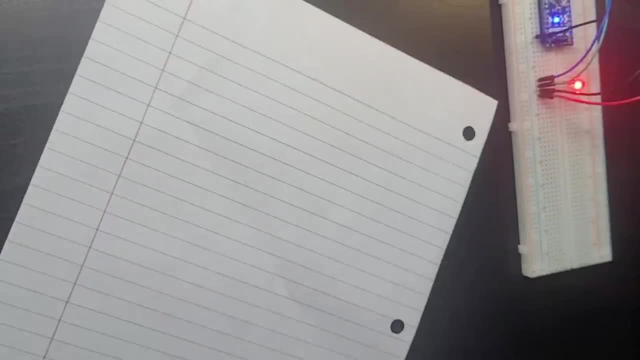 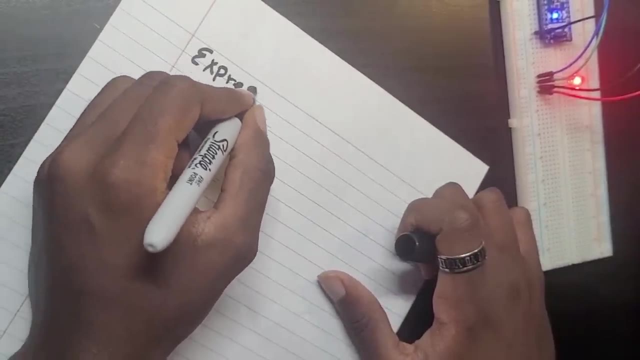 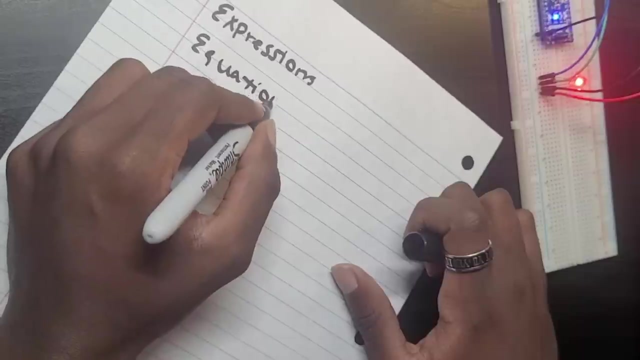 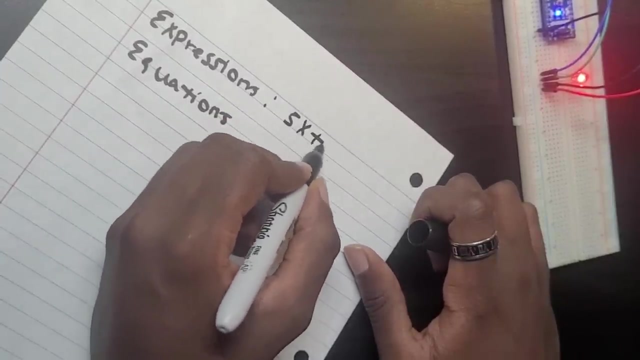 okay. so if you remember, if you guys learned about expressions and then equations, what is the difference right here? what is the difference right here here? When it came to expressions, all we have to say is what? 5x plus 7 is like an expression. 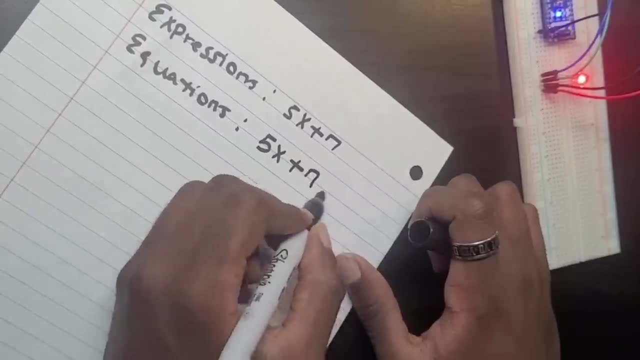 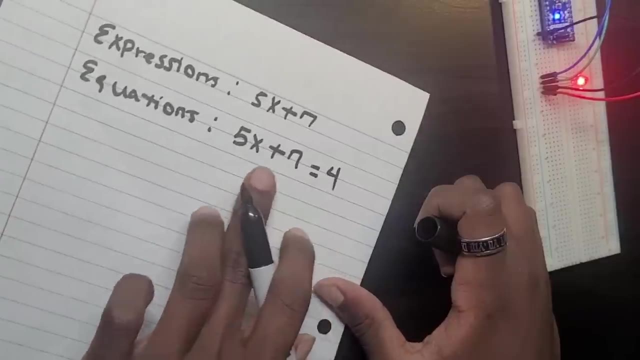 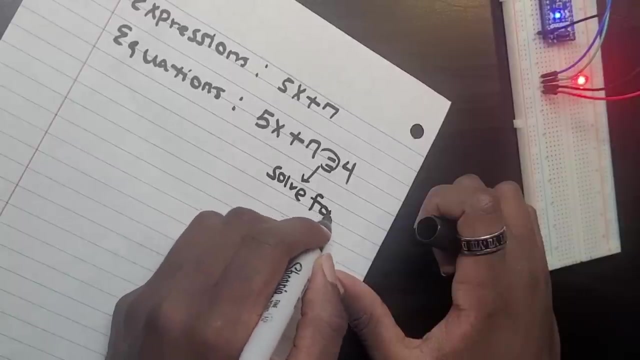 What is an equation? An equation has the equal sign. Let's say, 5x plus 7 is equal to, maybe here, 4.. Okay, So right here. what does this do? This means to solve? what does this mean When we set the equals to here? this means what Solve for x in this case? What if I? 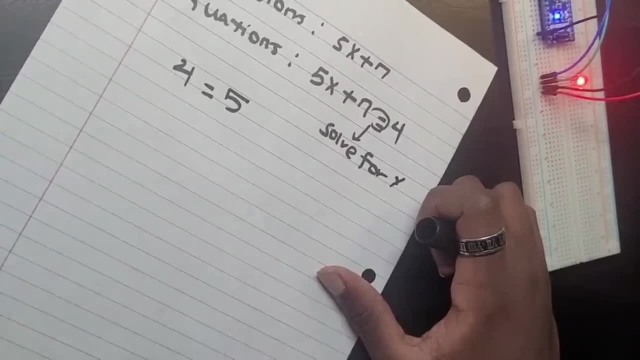 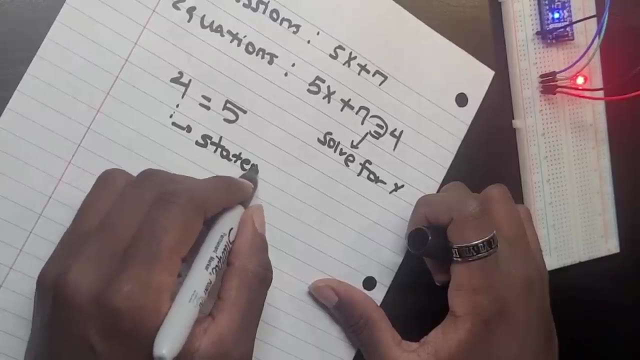 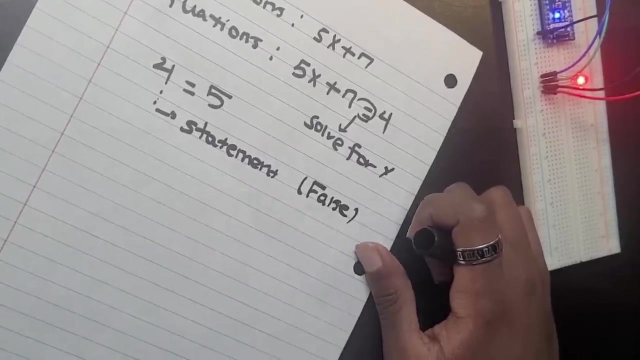 said: 4 equals 5.. 4 equals 5.. If I say that this is going to be what- This is a statement. And what is the statement? Is it true or false? This is definitely what. This is definitely a false statement. Okay, So we use the same sign right here to do what? To solve for x? 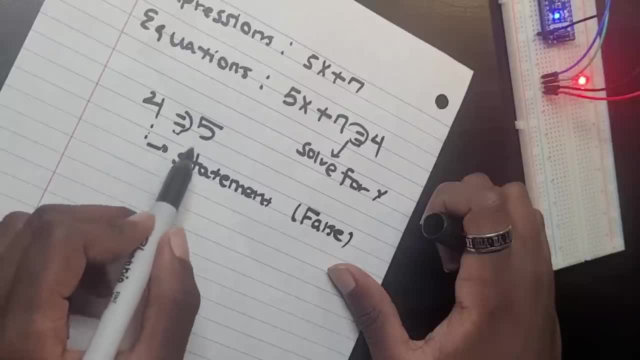 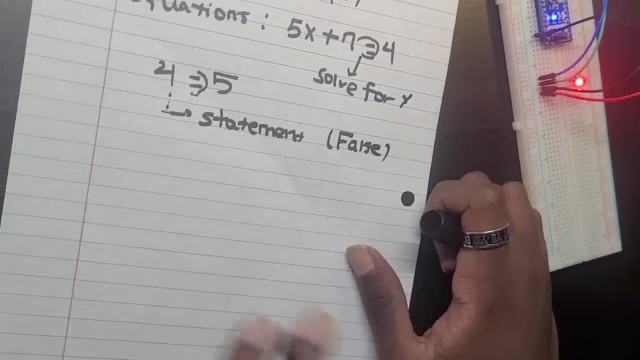 and what To even, what To see and compare and contrast. So basically, what We see, what The statement, To see, the statement. But When it comes to computers, I said that what Computers are, what Computers? take you literally. 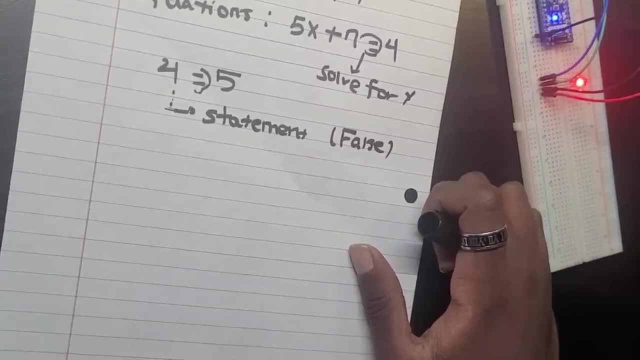 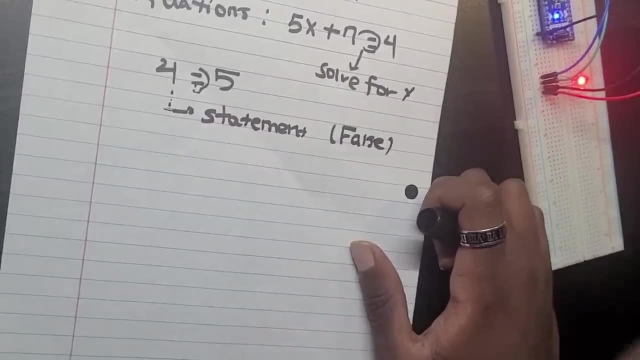 And I think all of you know that- That computers- what They take you literally, So they need to understand the difference between you are solving for x Basically. they need to understand the difference when it comes to computers right now. They need to understand the difference. 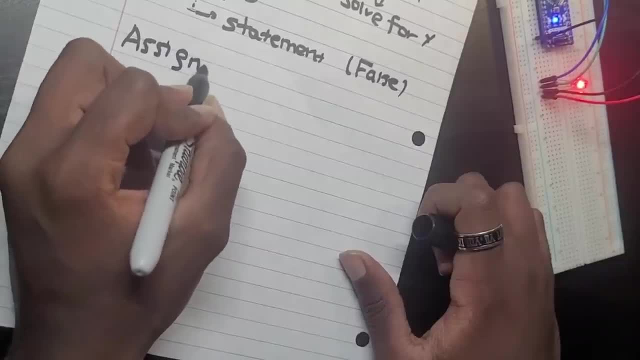 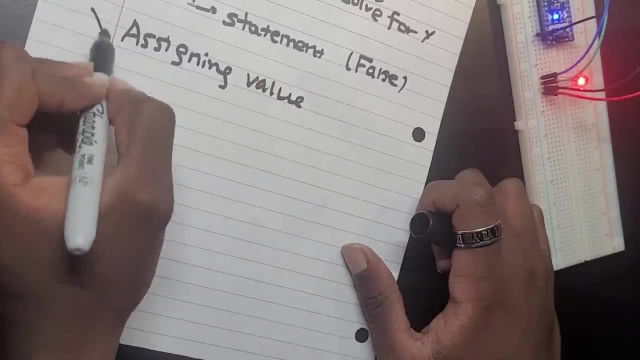 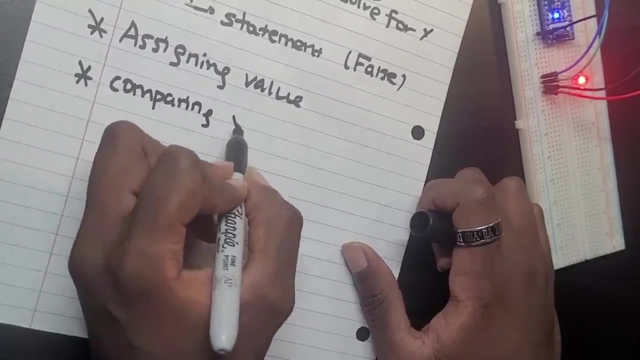 when you're assigning a variable, Assigning a variable, Assigning value, Right here To a what, To a variable. They need to know the difference between you assigning a value and a value and then you comparing a value with another, Comparing values, Comparing two values. 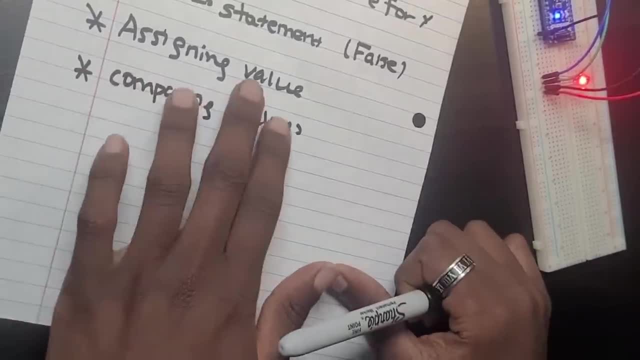 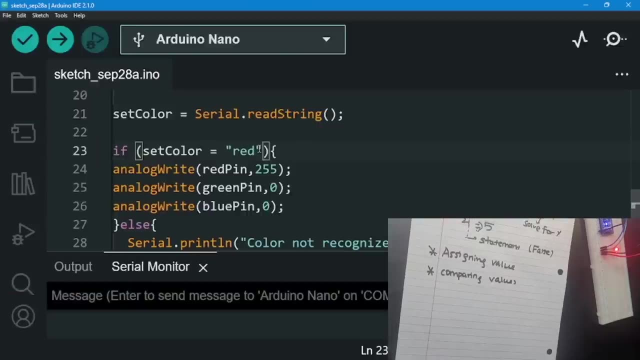 So how does a computer know when you're assigning a value and when you're comparing values? Because when we go to line 23 here, what are we trying to do? We're trying to compare the set color variable with what? With the string red If the string is equal to red, if the 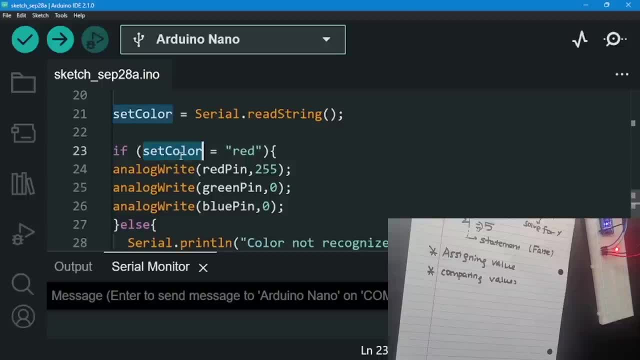 answer is equal to red. what are we saying? If it's equal to red, you want it to what? We want it to write what This code. It wants to run this code. We want it to run this code between line 24 and 26.. Okay, That's what we are basically saying, But it cannot know. 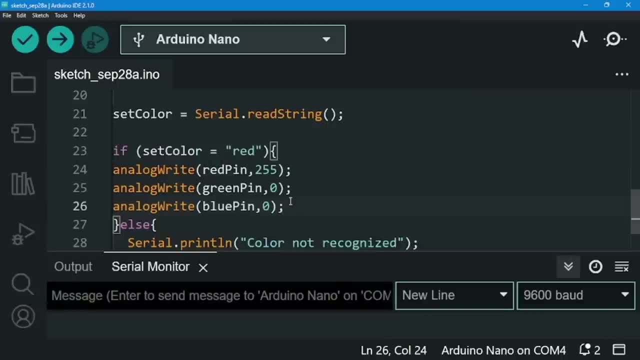 that. So, when it comes to assigning values, one thing you need to keep in mind is, when it comes to assigning values, you're going to be using the equal sign, Just like how we're using, again, the equal sign in line 21 to what To set the color Right. here we said: 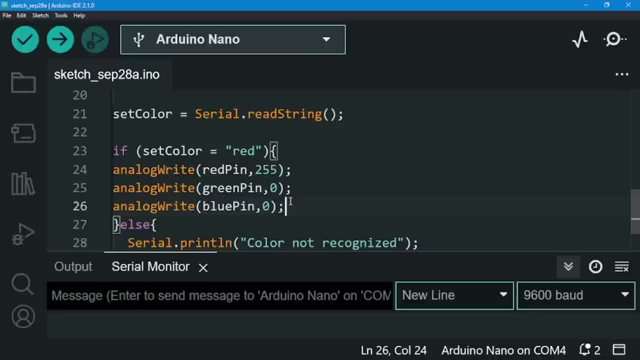 set color is equal to what Real dot? read string, The sign variable. See only what. Use what. We use an equal sign, But when we were comparing the values, what do we do is we use two equal signs- Okay, An equal sign next to an equal sign. When we do that, our Arduino knows that we're comparing. 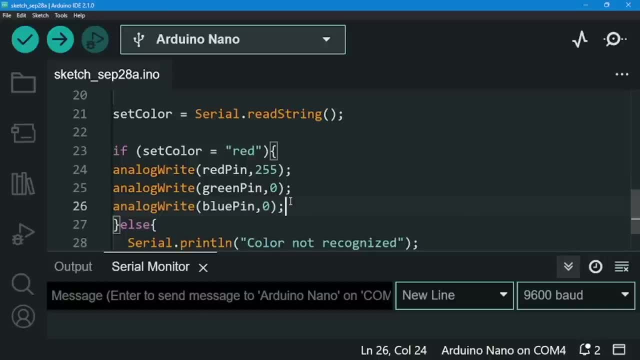 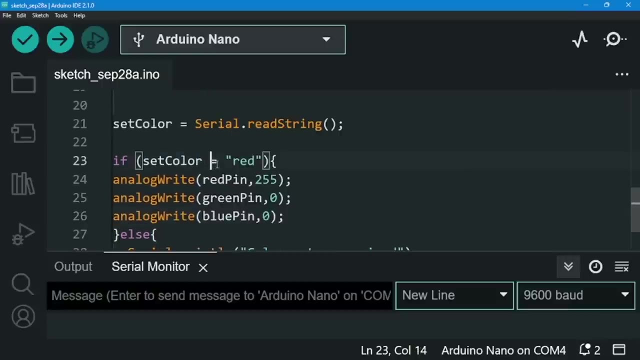 values. Okay, So we're not assigning values, We're comparing values. Okay, That's one thing I want you to know. Okay, So let me just move it right here and let me fix this properly. After what? Now I'm what? On line 23, I'm doing? what I'm literally comparing, what I'm literally comparing. 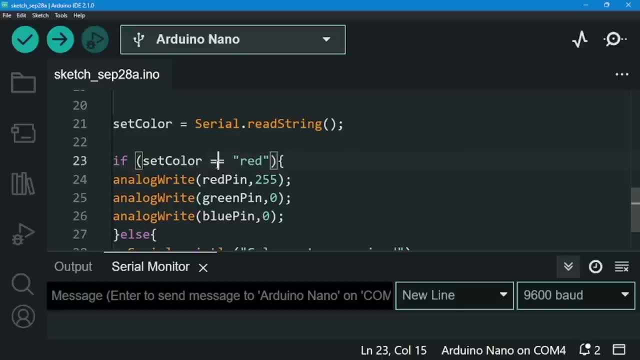 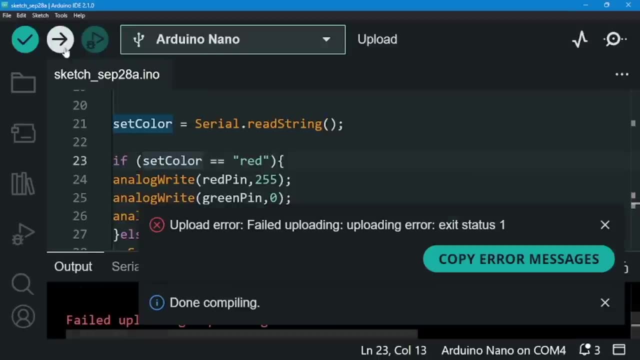 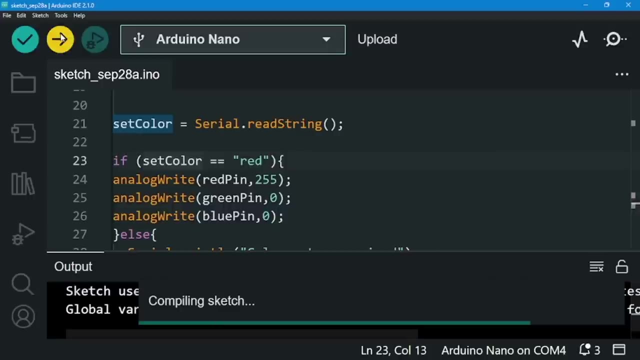 So what should I be using? I should be using double. There we go. I'm going to be using double equal signs here, And then let's upload it. Okay, I forgot to again close my C-Wave monitor. Happens often. All right, Let me go again. Should be uploading, Okay, It's. 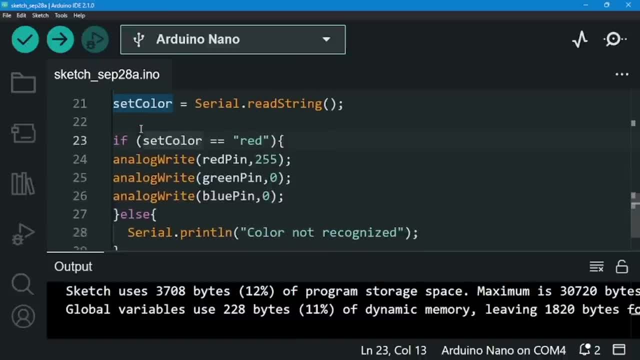 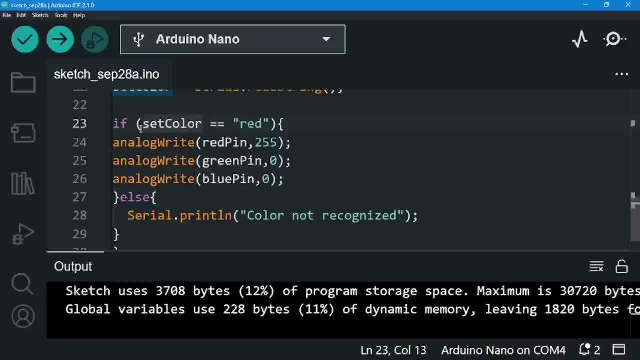 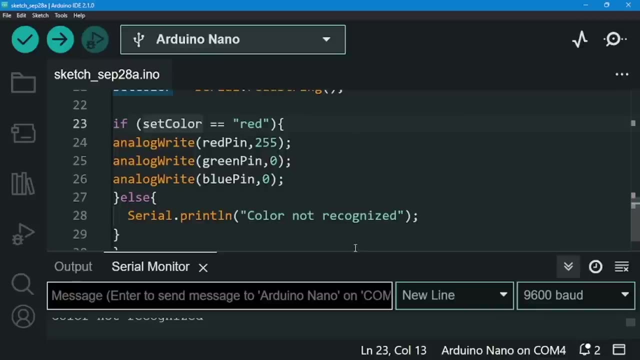 done uploading, There we go. Now everything is fine. There we go. It's not lit up right here, Okay, So now, what do we think it should do? right now, When I see red, we want it to turn to what. We want it to turn to red. So let me just do that right here. Actually, I 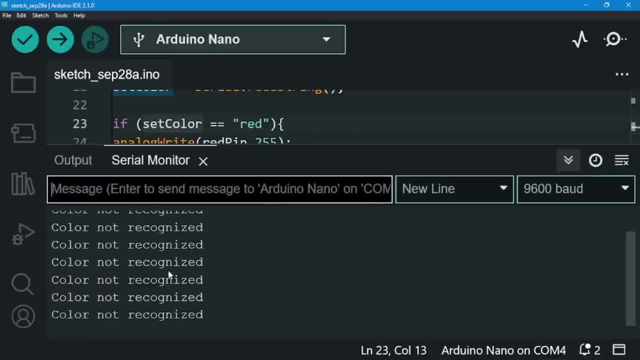 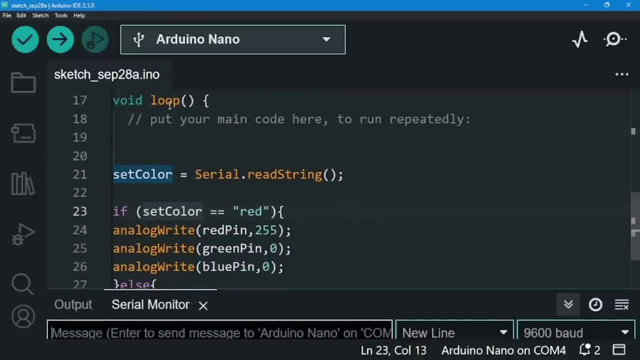 keep getting color not recognized, color not recognized, color not recognized, over and over again. Let's see why is this happening first. Okay, So obviously this is going in the loop right here. Right here it's a loop, the void loop, So it's going to check for. 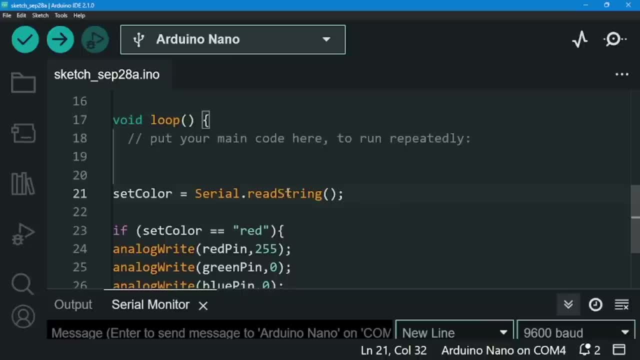 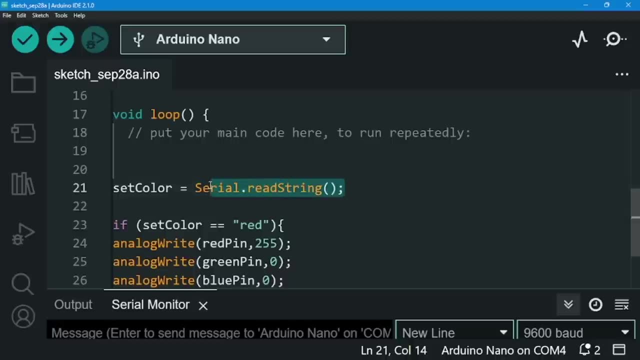 the set color. In this case I have not set anything, So it's going to be an empty string or almost zero, A zero or an empty string, Some somewhat like that, because I don't know about anything right now. Let's see what happens And then it's going to be checking for the 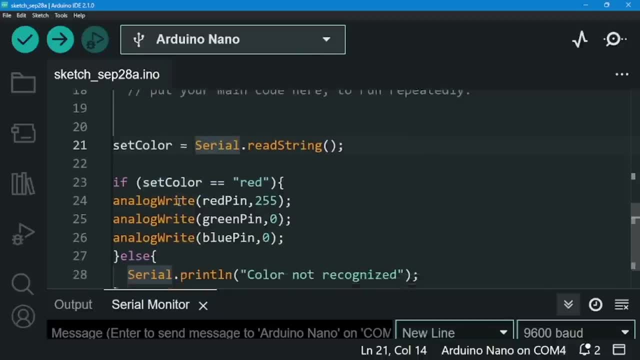 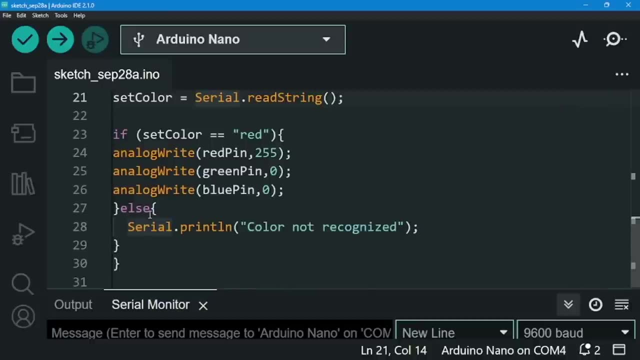 set color is equals to red. Obviously, it's not equal to red in this case. And then it's going to go: what to what? Okay, This is not true, So let me go to this one. Let me go to the else one. Okay, Let me go to the else one. It's going to say: let me go to the red. 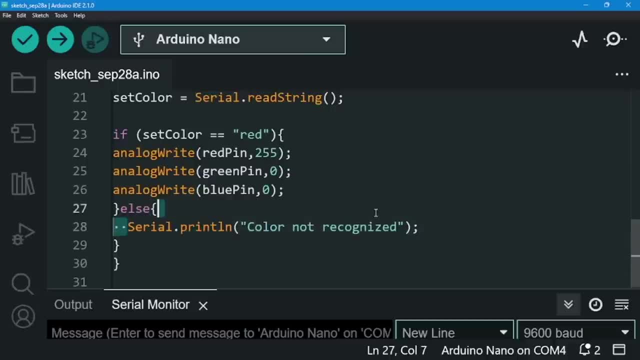 Let me go to the else one and do what And run this code again, And then I'm going to start the cycle again because we're in what? In loop. So that's the problem here. So let me remove the else for now, because it's quite, quite distracting for now. So let's remove. 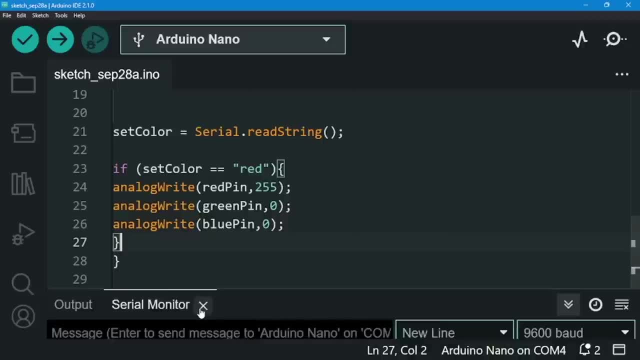 else, for now at least. So let me just turn off the serial monitor right here and try to upload it. Okay, It's done compiling and it should be uploading. All right, It's done uploading. So let's see if we're even going to run to errors right now. Okay, So let's. 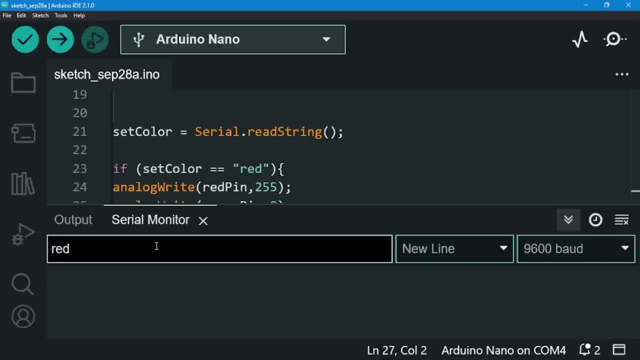 see So right now. when I see red, when I enter red right now, I expect this LED to turn to what? To red. So let me try to do that. I'm just going to touch the enter key right now And we can't see nothing. Let me try doing it again: We still can't see anything. 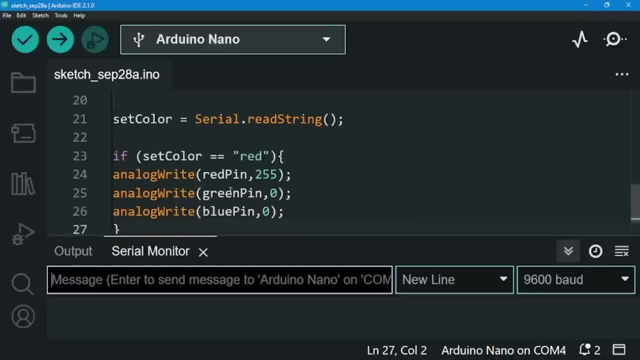 So in this case let me try to debug it All right. So one way to debug it is what? Let me go to my serial right here and say: serial dot, print it. Let's try to print the serial Set color If there's even a problem with it. So let me just check if the set color 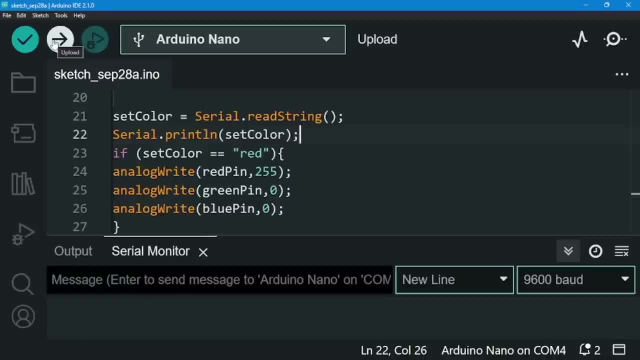 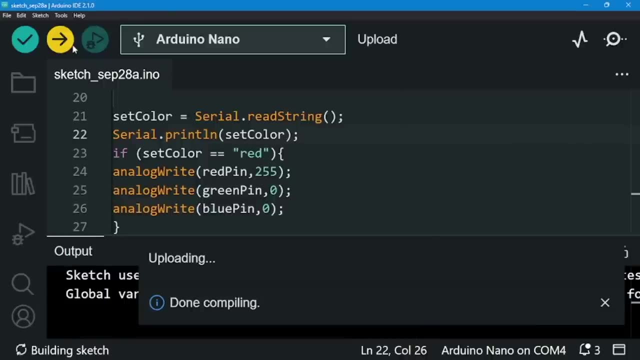 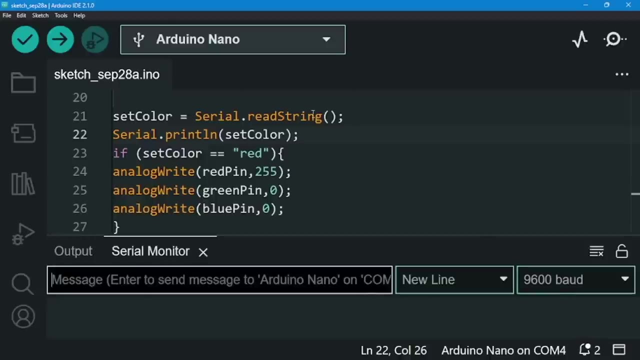 is correct. So let me just upload this. But before doing that again, turn off my serial monitor. Let me just upload this right here. It's done compiling. Okay, It's done uploading. All right, Now let's try to go to my serial monitor. And now let me try to go to my monitor. 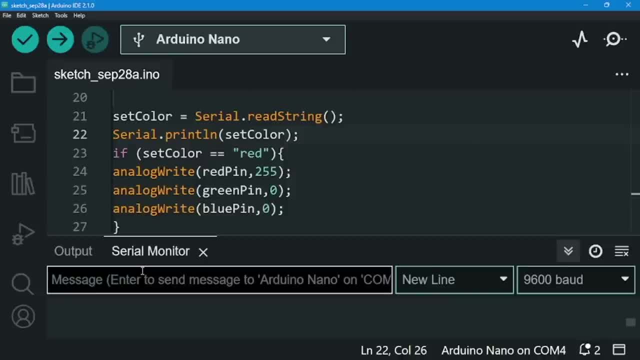 right here. Let's set the value to red. Okay, All right, So now it's done. So I'm going to do that. Okay, Let me just try to do that. Okay, It's not setting to red, As you can. 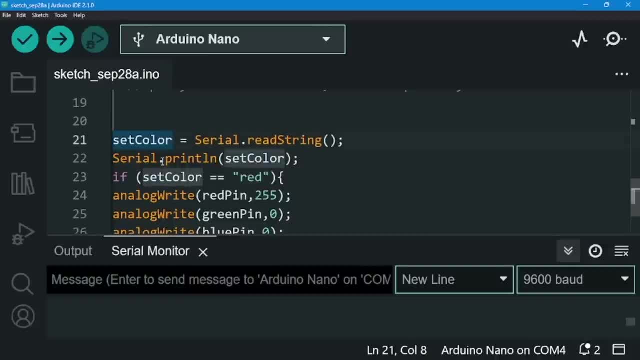 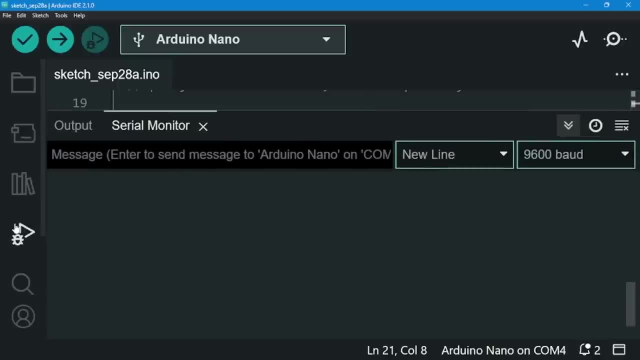 see right here. what is the problem Again, what happens? It's just printing out, I think, an empty character. There we go, It's emptying out. Look at it, It's going down and down if you look at the pointer, But it's emptying out. what? Printing out empty characters? Why? 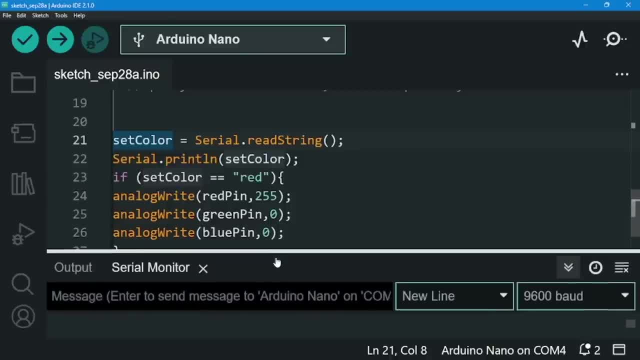 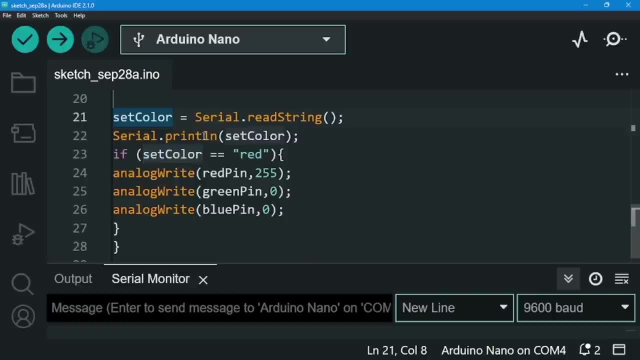 is that? so I don't put anything inside of the message. again, I don't put anything inside of the message, For instance, I only put what? Red, for an instance, And then it keeps running and running and running again. So I need to put it where I need to put this, the print one I need. 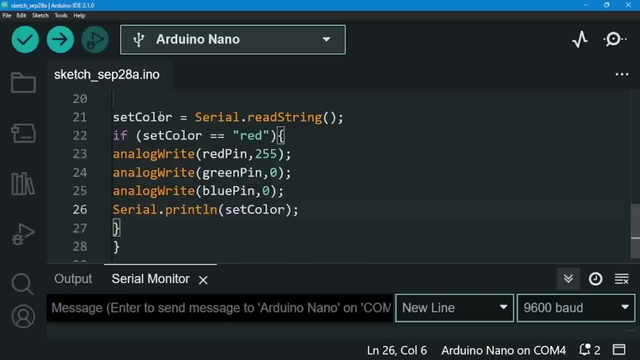 to print. put it right here: I want it to print as soon as what It turns to red. I think it's better that way. But it might not even print it. because why is this a bad idea? again? Because if obviously this is true, it would have run this, So it always skipped. 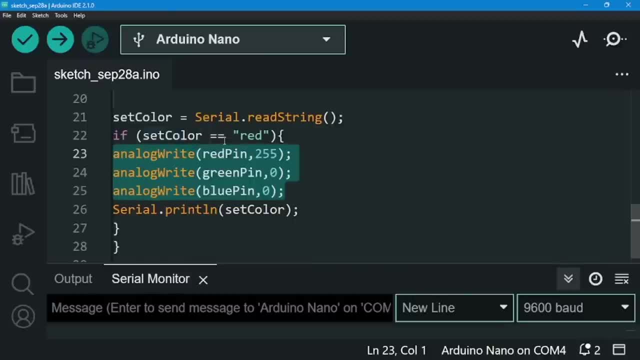 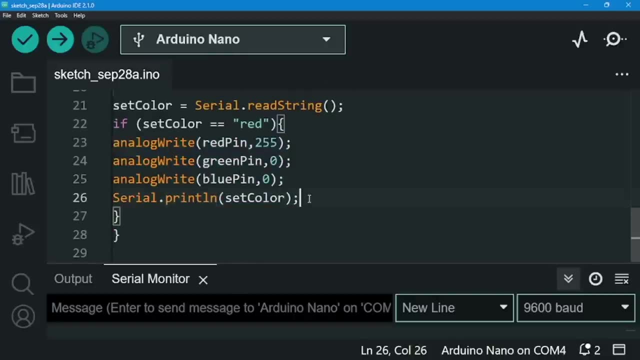 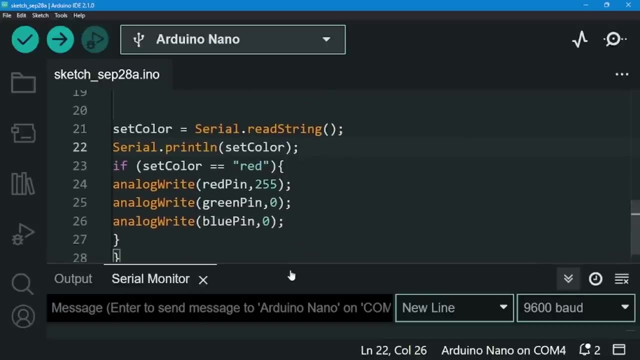 this. This basically means it always skips it. It's saying that set color is not equal for some reason, And I need to figure it out myself. So let me try to do is let me try to do is just go over here Before the color right here. What I want to do is I want 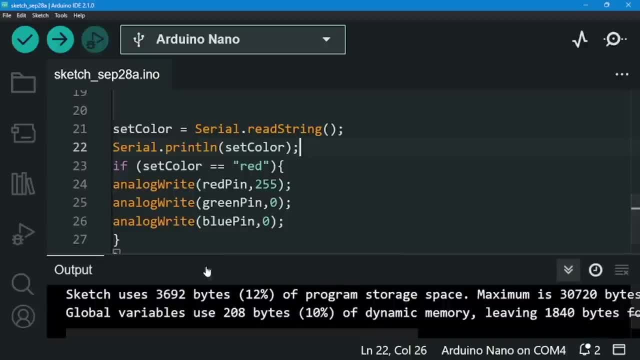 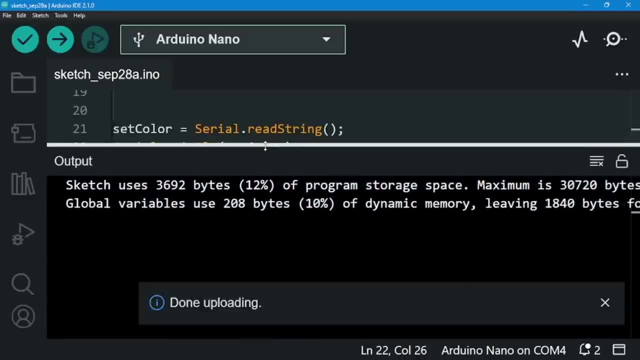 it to read the string and then, okay, let's try it again. It's better that way. Let's try to see it, because it's really hard to work from here. Okay, Let me just do that. Okay, It's done uploading, So let me try it again. Let me try it again. Let me try it. 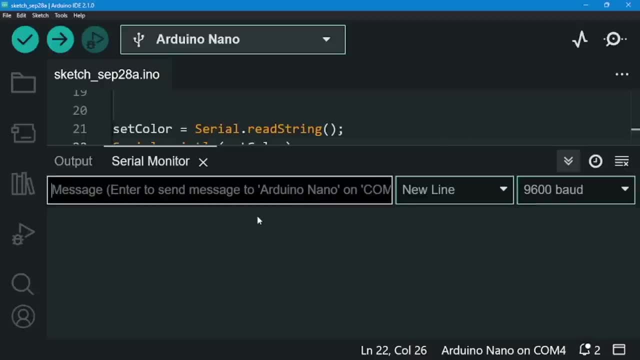 again. Let me go right here. Let me just say red. Okay, There we go. There's an instance of red right here. Before I get it runs through it, Let me forget about the no line ending right here. Let me focus on the red right here. There we go. Can you see it? The red. 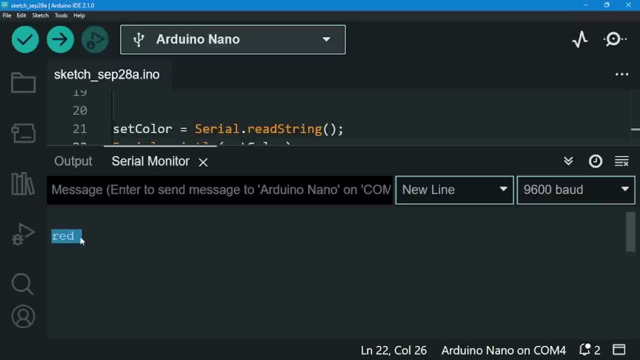 has a what right here, It has a space. Can you see this? It's like writing it as what Problem here is? like a straight component of writing it as what? As a red, And then maybe you're putting a new line. 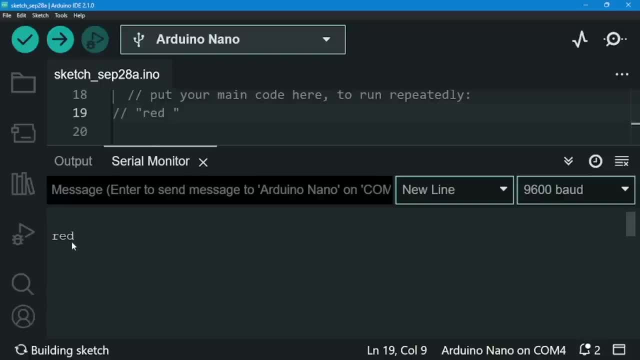 Right here you're giving it a space. It looks like this because it has what They said. again, it has a space next to it. So obviously, this red is not equal to what It's not equal to, not equal to what, To the red we have again on the color right here. 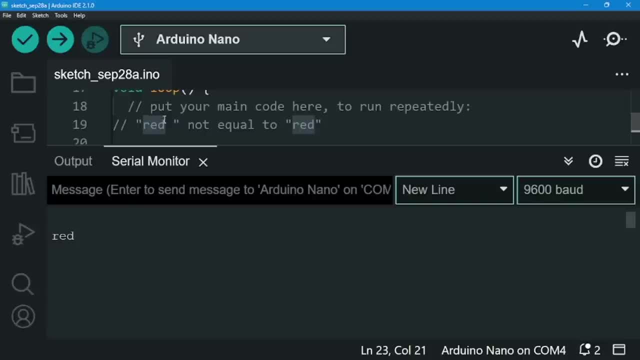 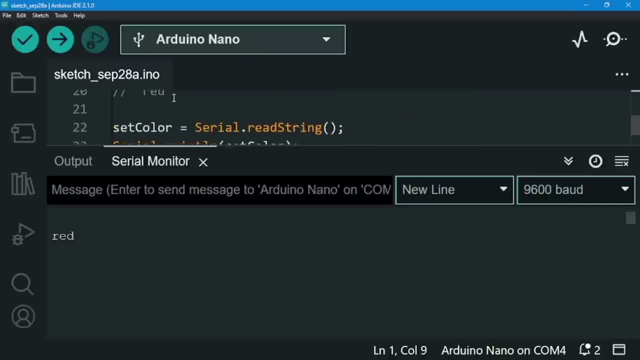 Right there It's a space or it's a new line, because I can not extract that information right now- Can be a red or it can be what? A new line. right here, at the end, At the very end, there's a new line. It's creating a new line here, Okay, So let's see if it is a new. 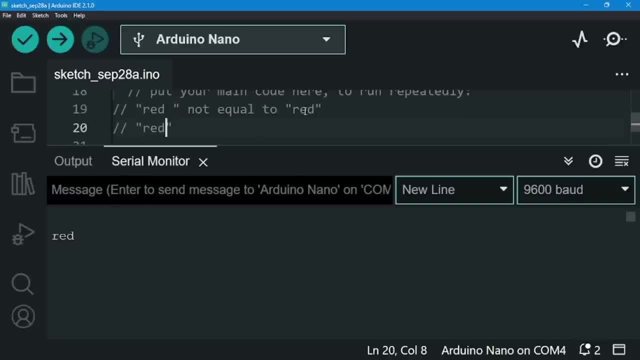 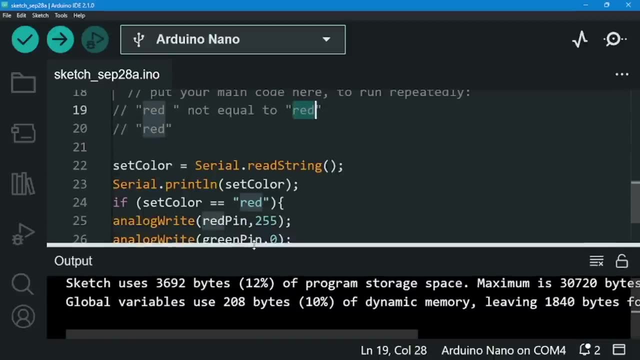 line or just a space, so that we can adjust it to what we can adjust the our red right here, The string that we have to again compare it to. So what I'm going to do right here, it's going to be a. you know what, If it's a new line, I should print next to it, I should 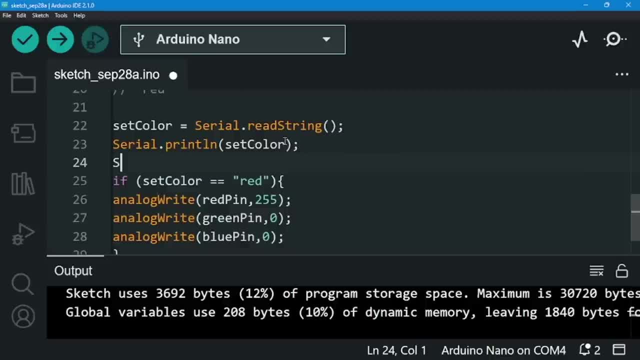 be printing something next to it, so let me just print something next to it. print, not a new line. let me just take off the new line right here. let me just take off the new line from both codes and if it's a new line should basically what this: 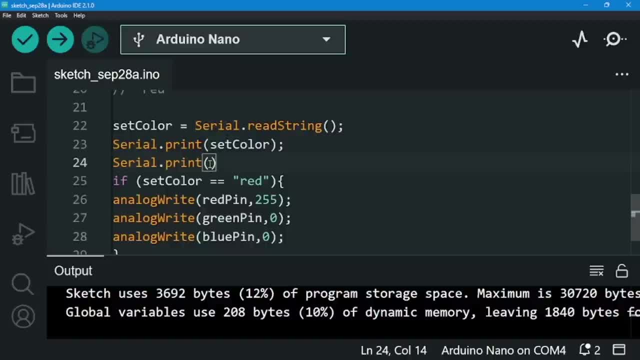 one should be on its separate line again. so let me just print out maybe, then say hello, okay, hello, or hello, there we go, there's that. so basically what should happen right now? if it's no, if it doesn't have a new line or space, what happens? let's see what's gonna happen. the two scenarios: the first scenario is: 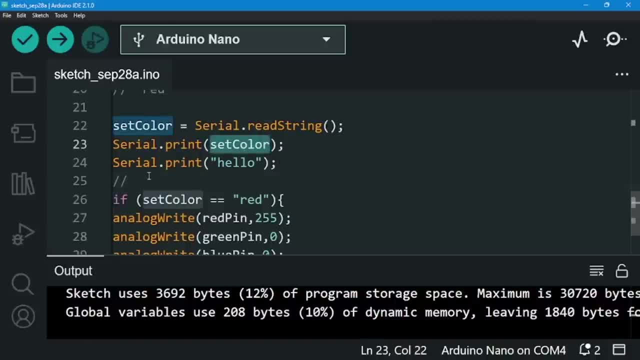 what? the set color, what doesn't have any string. so basically, it's gonna appear as what is red. by the way, for those of you who have a legacy version, it's gonna appear. it's gonna work for you guys. okay, I'm gonna get back to you guys, so right. 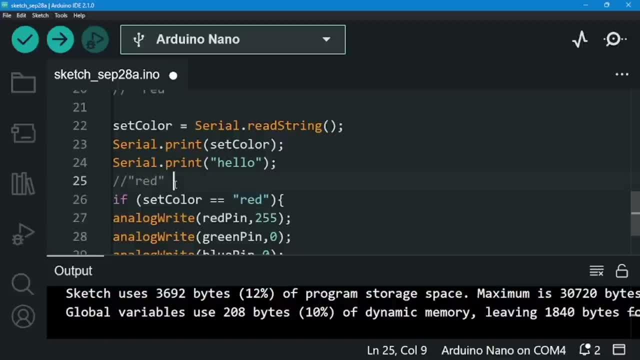 here red. okay, it's gonna appear it's red or we're gonna be receiving what we're gonna be receiving: red with a space. as we saw on the serial monitor, it had space when I selected on it and then, or it might be a what, it might be a red and it has a new line at 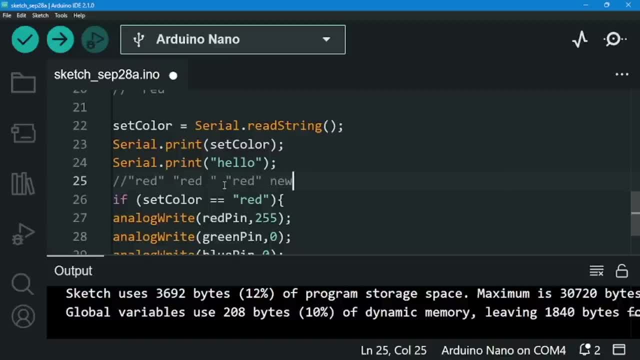 the very end it tries to make a what a new line. just write that a new line. okay, that's what it's trying to make. so how do I know if it's a new line or a space? I received a one that had what again? a space right here. how do I know it's a? 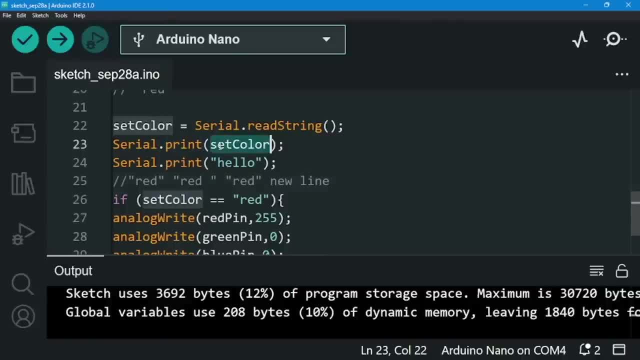 space or a new line. obviously what I do is again put a hello next to it. so if it, if it doesn't have a new line, what's gonna happen? there's a space right here, what should it give me? should give me, like red right here. say after the space, say hello, okay. but if it has a new line, on a new line, 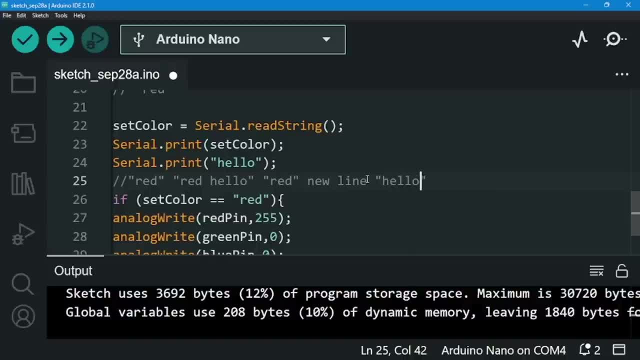 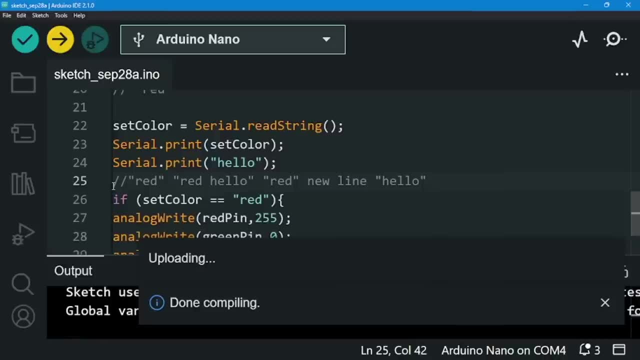 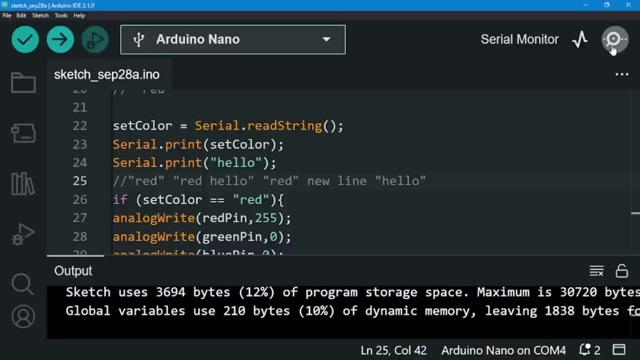 on another line we're supposed to be receiving what? hello on a new line, on a totally new one. so let's see what happens here. let me just upload this again. so again we might need to what you might need to adjust. again. this makes no sense, as I said, again, it makes no sense why Arduino is doing this, but again we 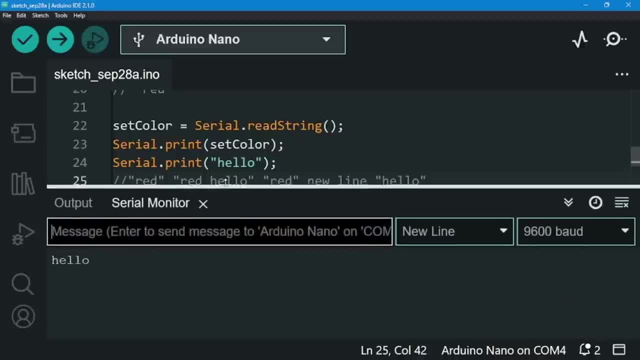 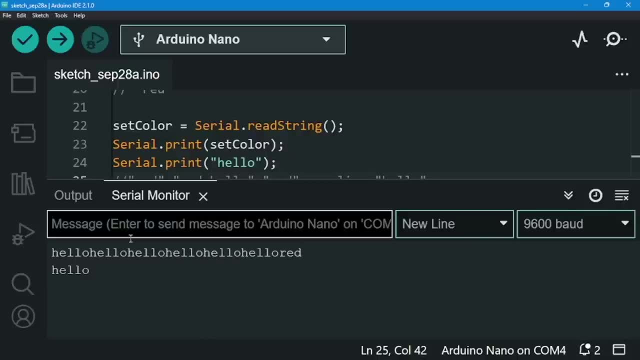 just have to adjust. okay, so it may also mean that we're already archiving something like something really gonna need to lighten a little bit. yeah, all right, there we go keep saying hello, hello, hello. now let me try to say: red right here. look what happens. there's a red right here and at the very, and look what happens, right, 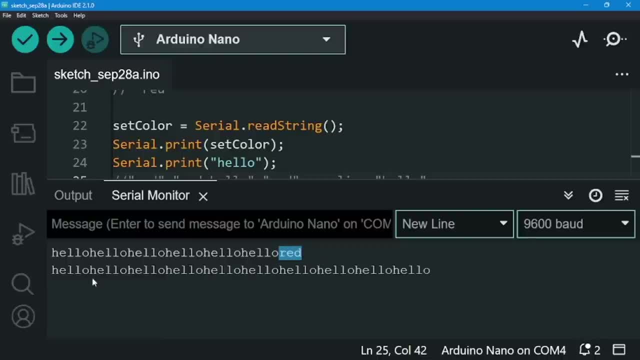 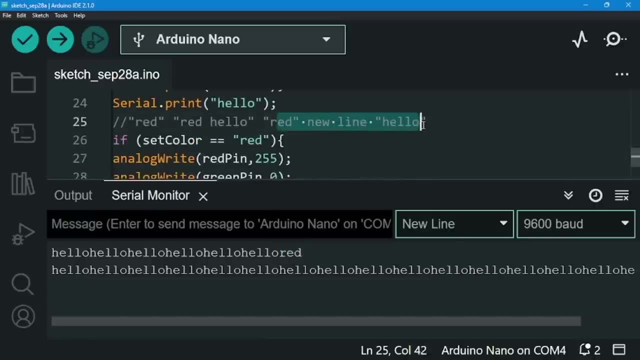 now, when I even go to the very edge, there's no space right here, but it pushes this to a new line. so what does this mean? this means that what we're having? a red that is attached to a new line. so one thing that we have to know is what when we're using serial dot- sorry, serial. 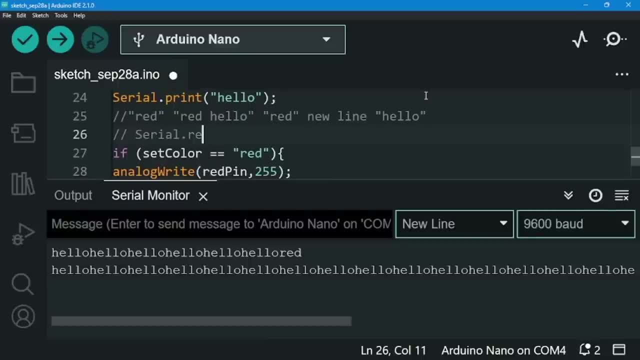 dot print. sorry, what was it called? restring read string. okay, when we're using serial dot read string, one thing you always need to keep in mind is what it prints out. strings prints out strings, okay, and it prints it out. and what prints it out in a new line? okay, all right, that's one. that's sort of the two. 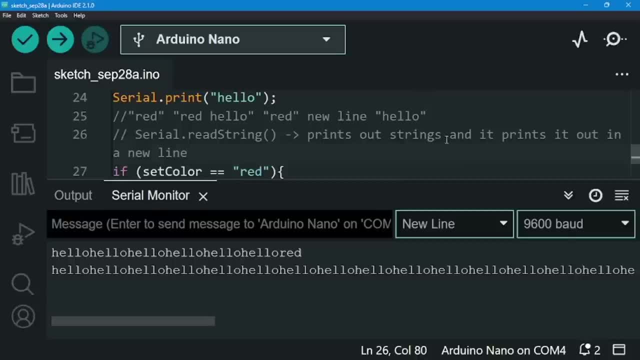 things you want to know. okay, prints it out in this, in the string, and it prints it out- and what in a new one, one other thing too- and prints it out in the string. so one other thing I really want to show you guys is all right, let me just 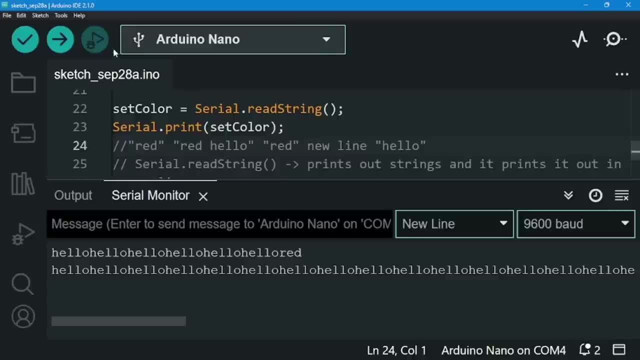 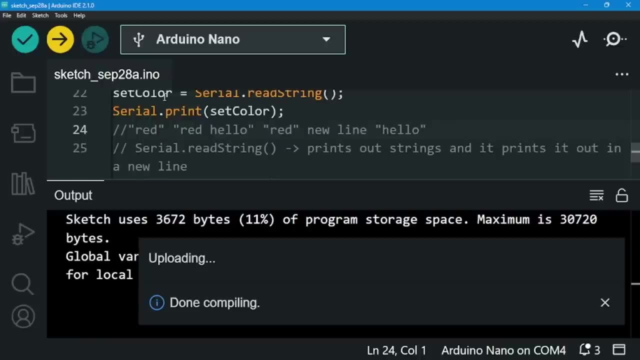 remove this hello right here, so that it comes, becomes really easy to teach you guys this one. when I mean that it prints out everything in a string, I'm actually gonna show you what, whatever what I mean by that, okay. so right here, let me just right here. okay, if I write down 10 and if I print, 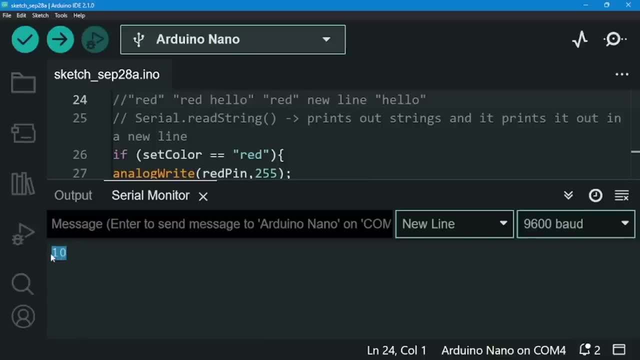 it out. what's gonna happen is it's gonna give me a version of this. so what I have right here, what I gave our do you know, our do we know, is what the number, what they give it the number 10. I gave it the number. it's a number 10. give it the. 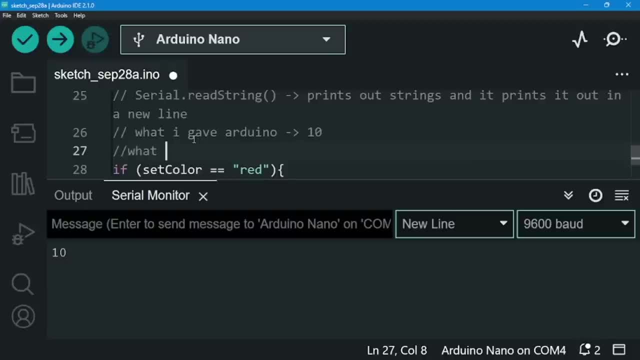 number 10. what did our do we know? give me what our do we know? printed again, what Arduino did get set serial. sorry, let's sell what color right here. what was my variable? thought Reno set color again. what did it set the variable again to is listen, it set it to a string 10. okay, a 10 inside of a what? 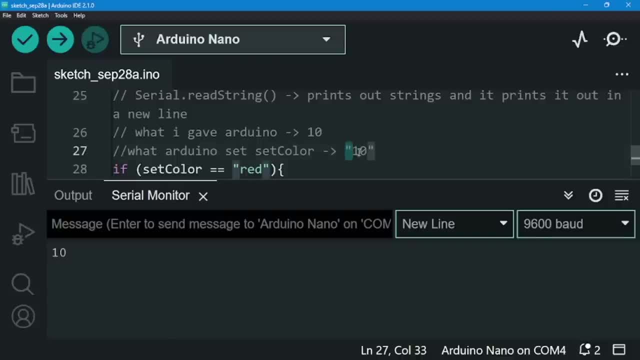 inside of a string. so what? this is basically me. okay. one thing I want you to understand here is: it looks quite the same. don't you look at it, doesn't look quite the same. one thing I want you to understand here is: it looks quite the same. don't you look at it, doesn't look quite the same. 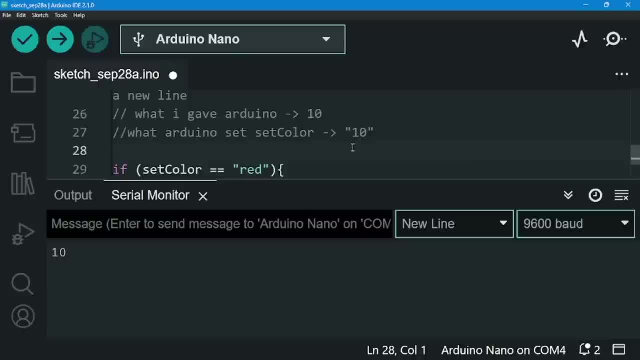 but it does not behave the same. Why is that so? Because if I said right here, if I said 10, let me just say 10 plus 5, and just write it down and let me just compile it- I'm not going to upload it, but just compile it right here. 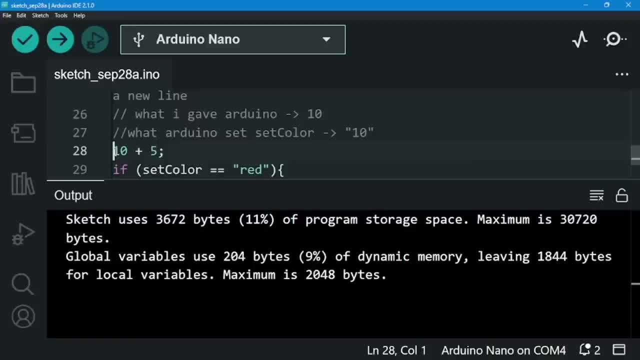 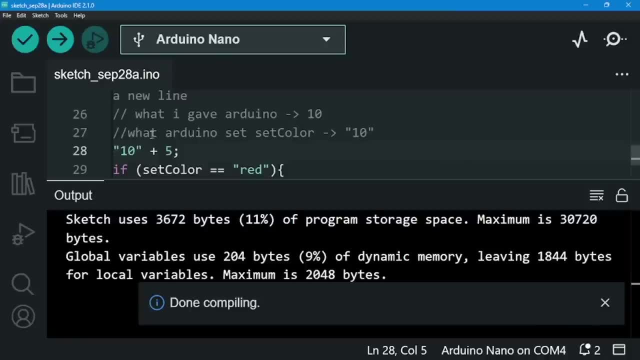 I'm not going to have any sort of error. But if I just do a string version 10 right here, get a string 10, and try to add it up with 5, if I add it up in 5, it doesn't seem like there's a problem. but if I print it right here, 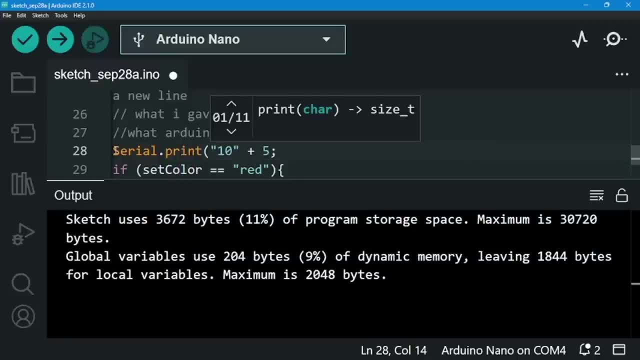 let me just print it. print this and a new line. Actually, I should be printing it in a new line. Let me just print this in a new line, Let's see what happens. Let me just verify it and then let's upload it. 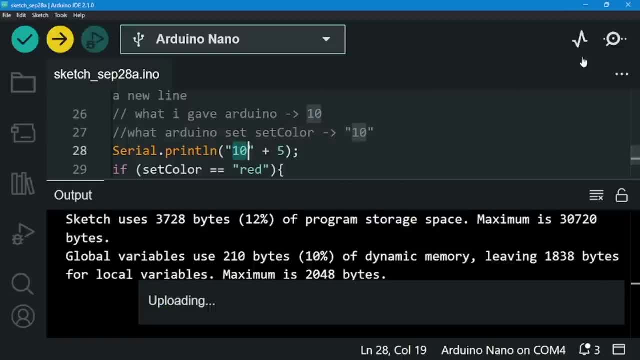 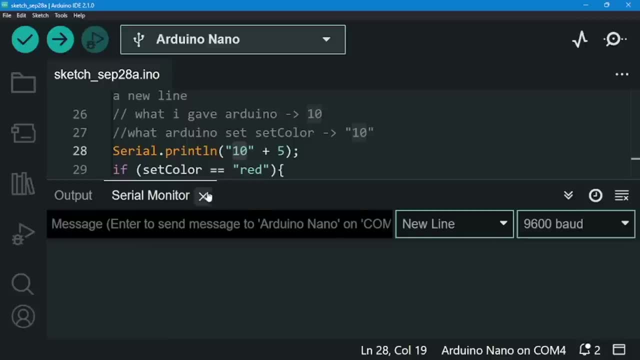 Let's see what happens when I add up the string 10 with 5.. Okay, so as soon as I open my serial monitor it says confware is already connected. Okay, let me just get back Here. let me try to unplug my Arduino. 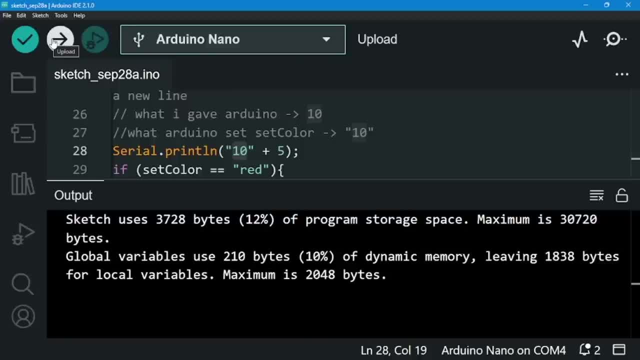 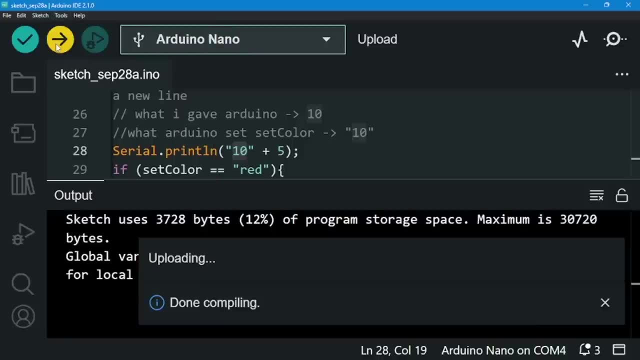 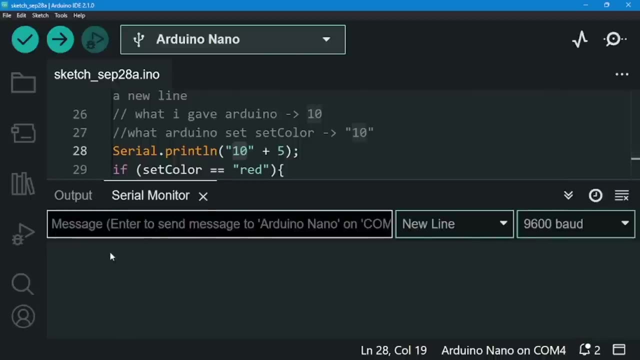 and then let me plug it back in. Okay, now I think it should be working. Let me just try to upload it. Okay, it's done compiling and I think it should be uploading by now. Okay, So when I go to my serial monitor, I should be getting what 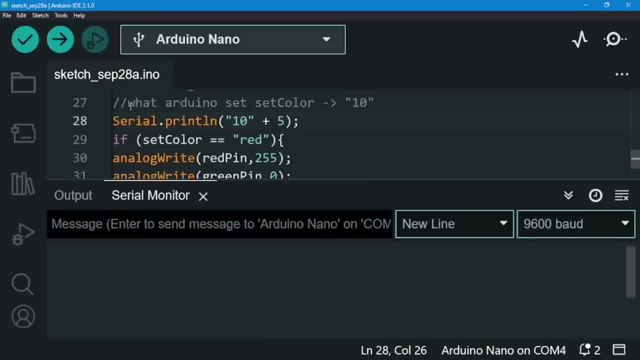 I want to see what happens when we add up 10 and then 5.. So let's see what happens when we add up 10 and 5. It's not printing anything. Let me just see if it's even capable of printing something. 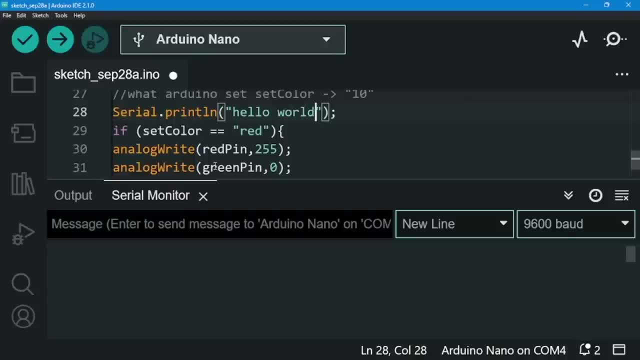 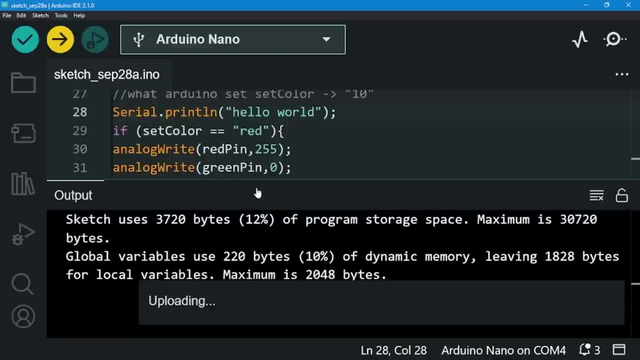 Let me just say: hello world. Okay, let's just save that. Let me try to upload it. Take off my serial monitor and it's done uploading. Okay, It's not Okay, there we go, Give us hello world. 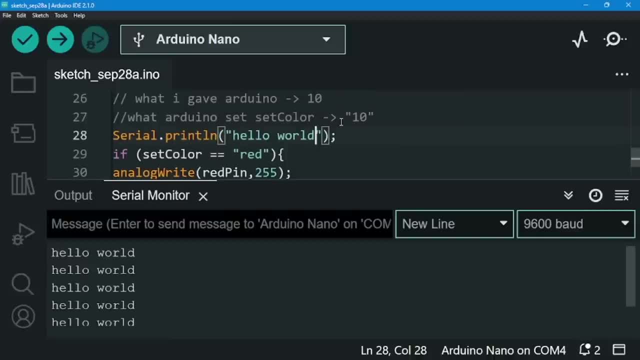 There, There we go. So what I'm going to do is you know what? I think it's not going to add it up. Let me just say 10 right here, And I think it's capable of adding it up. Let me just go right here. 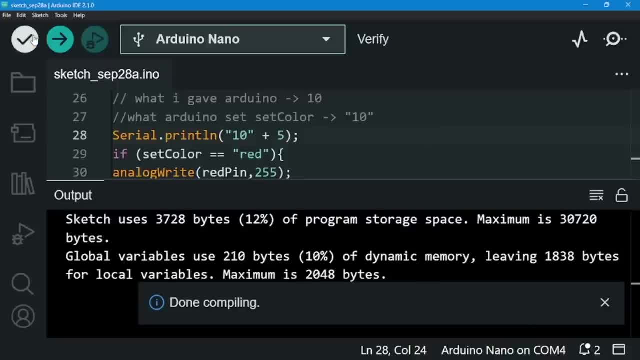 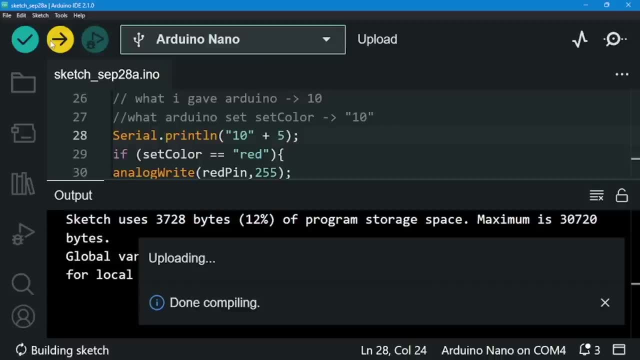 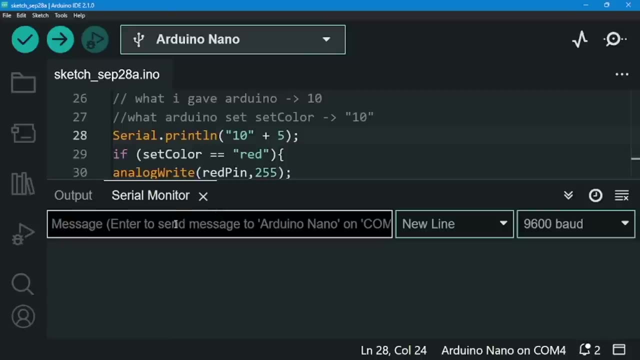 And let me just verify it. Okay, it's done compiling, Let me just upload it. Hopefully it won't go into an error. All right, nice, Now let's see what happens. I'm still not receiving anything. Can you see it? 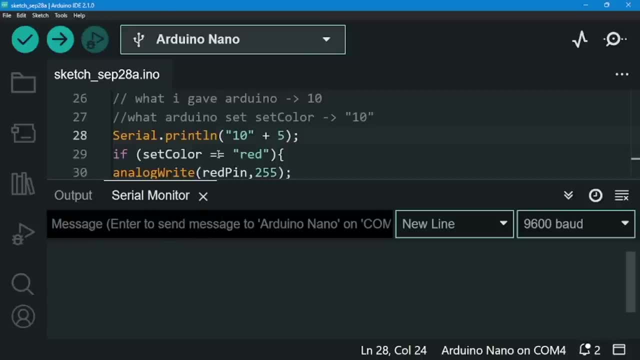 You're not receiving anything. But basically what happens is we cannot add what we cannot add. Can you see? we cannot add strings. to what? to numbers? Have you ever thought of adding up a number to a text? I don't think it's even physically possible. 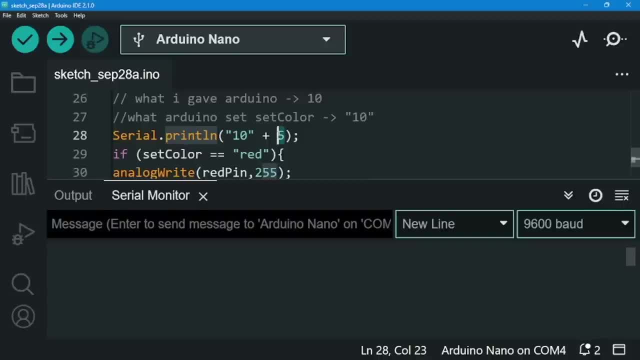 You know, we cannot even do it. theoretically It's not possible. Obviously it's what it's sorry, does not obey the law of math. Obviously we cannot do what. we cannot add a text to what, to a number. So basically we cannot add a string to what. 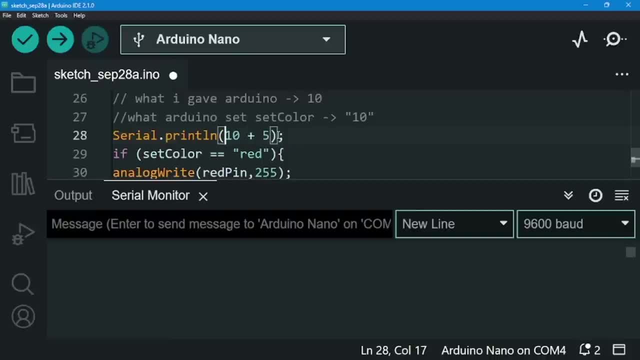 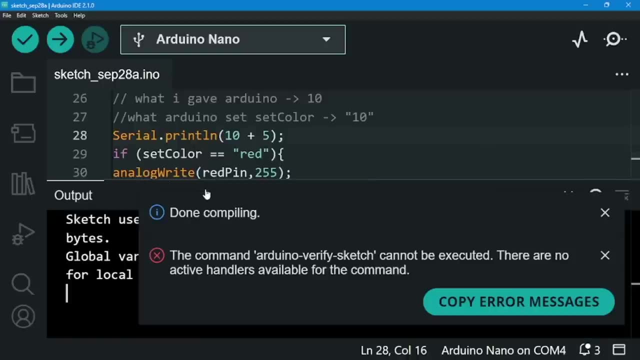 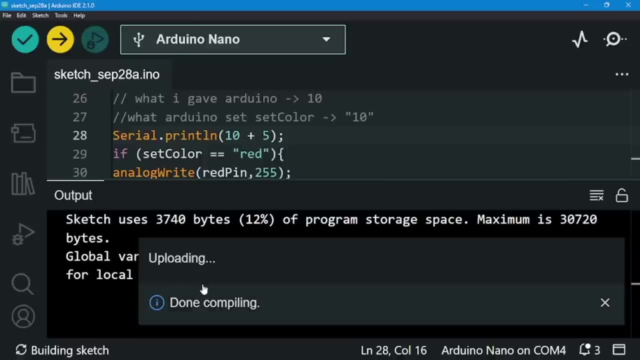 To a number. But if I see 10 plus five right here, 10 plus five, and let me try to verify it And let me just try to upload it. How about now? Let me try to upload it. It's done compiling and it's uploading. 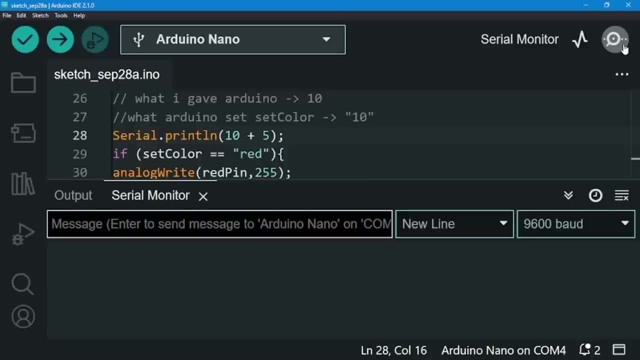 All right, it's done uploading. There you go. It starts to give me what? the number 15, the number 15, the number 15.. 10 plus five. So that's one thing I want you guys to keep in mind. 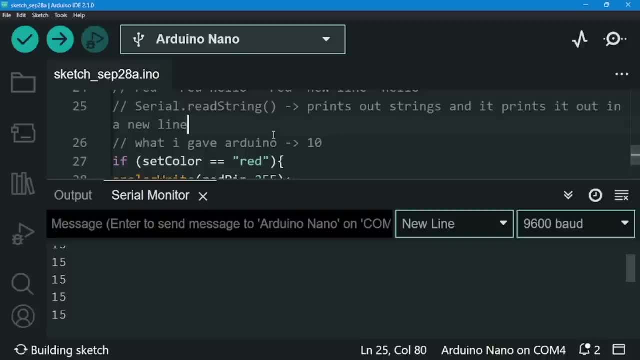 Okay. so when you're working with, when you're working with again those serial dot restrings, what do they do? Their name even gives us away. What do they do? They always convert anything. They print out strings every time. 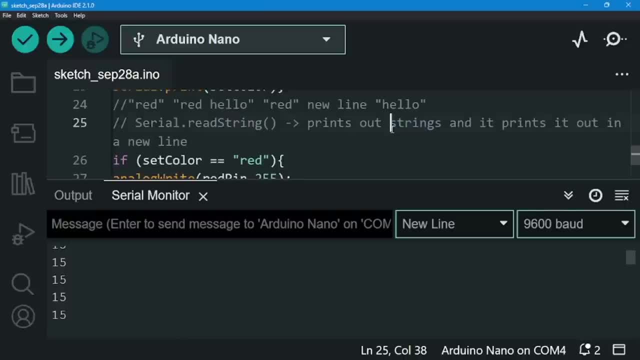 What they do. they always what. When they store values, they want to put them in strings, And what they do they print it out in a what In a new line. Okay, All right. So one thing you need to know before actually you know working with. 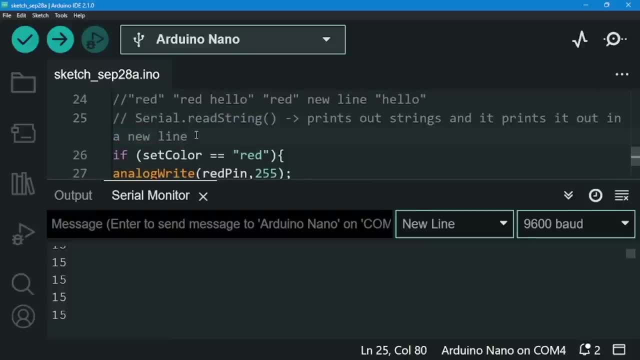 this, before actually finishing up, is what we need to make it. so we need to create a new line character. We need a new line character so that it matches what this one right here. Right, Because right here set color is what Set color is, not only what we set as a string. 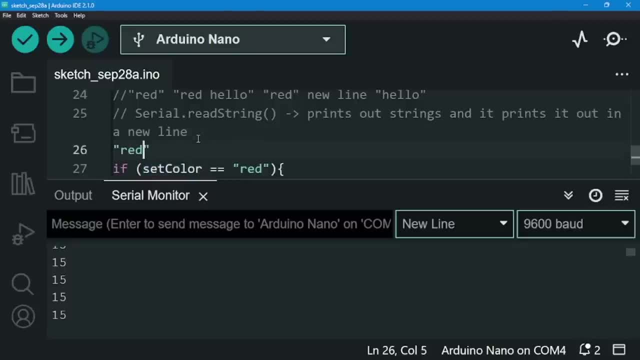 What does it also have? It has a new line. It has a new line. Okay, So it's not going to be equal to. it's not going to be exactly equal to what. To red Again. if it was a human being, it would have understood. 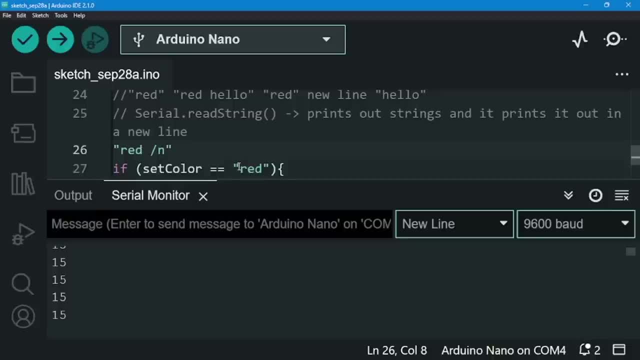 Obviously it would have understood that these things are equal. But when it comes to computers, again, they take it what they take it literally. So it has to be literally equal. If it's not literally equal, it's not going to take it. 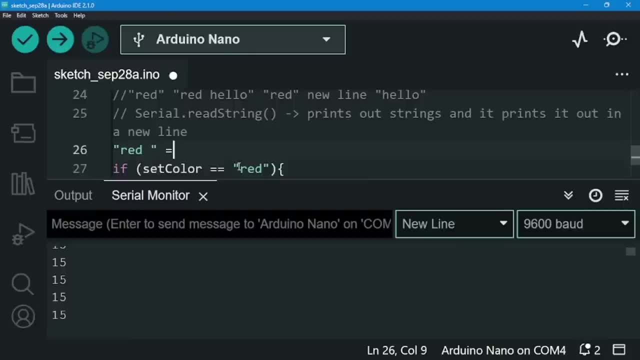 If I said red like this, with the space is equal to red, it's going to say it's going to give me the output of what. it's going to give me the output of false. Okay, It's going to say it's false. 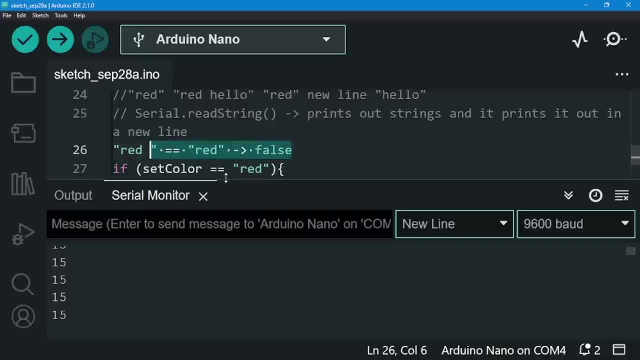 It's not true. But obviously, if it was a human, what would they say? You say it is true. Obviously, as we can, we can account for mistakes, But computers, again, they take it what Too literally. So with that in mind, 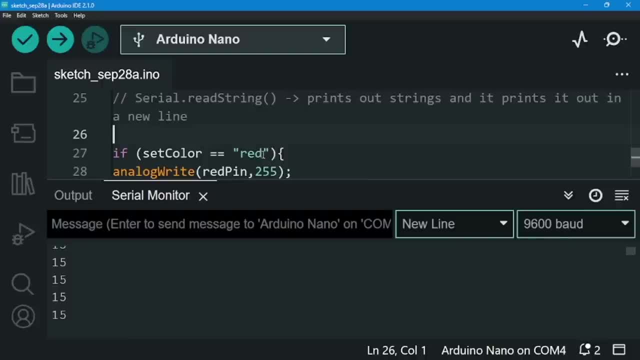 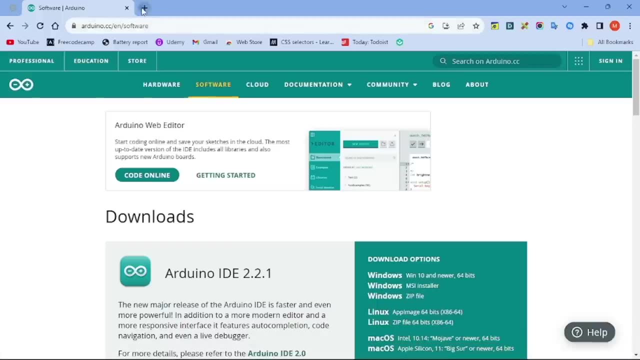 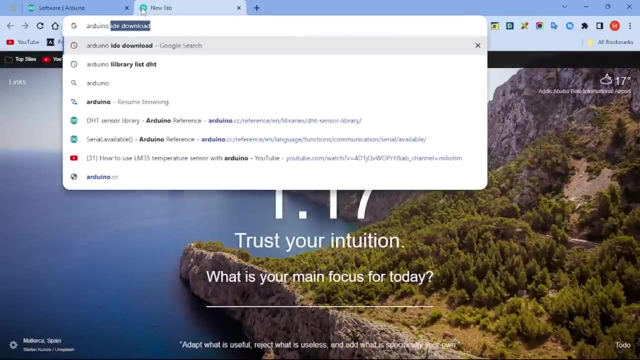 How do we represent the new line characters? That's the big question. This one represents a space, But how do we represent a new line? Well, if you go and Google right here, just Google it right here. If you go to slash n, okay, slash n. Arduino new line. 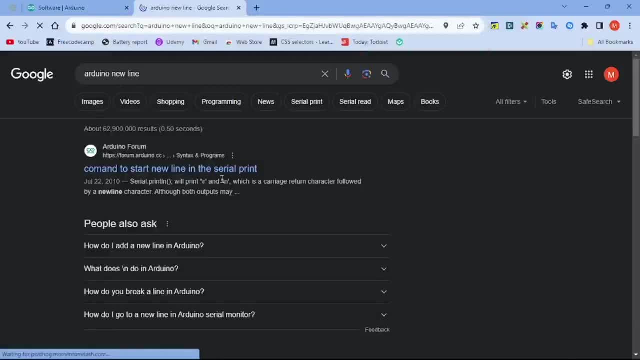 If you see Arduino new line, it literally starts with a. what With a backslash n? Can you see it? It says slash n. There we go, Slash n, Slash n, Slash n. Okay, That's one thing I want you guys to understand. 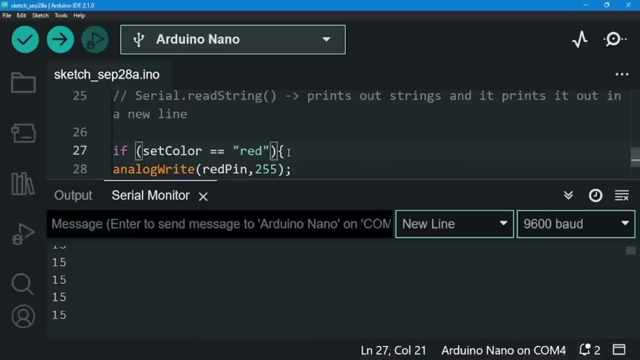 Slash n. So what you're going to be using is a backslash, So it's going to be beneath your backspace or above your enter key. So there's a backslash and there's a forward slash. Okay, Don't use the one. that is what. 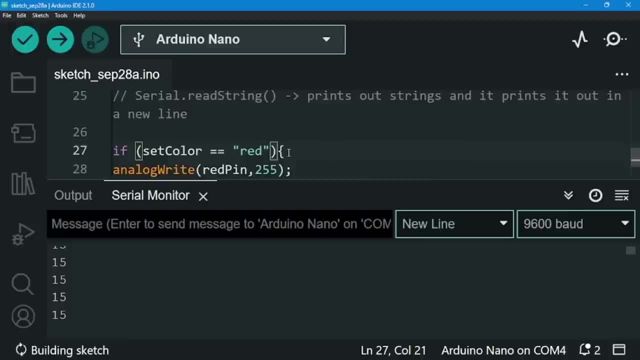 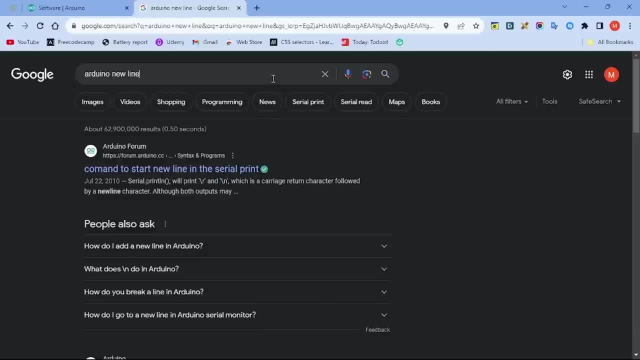 A forward slash, Use the one. that is what Backslash. Okay. So even though let's say you do not have that character, even on a keyboard- let's say, for example, using an old keyboard and you don't have that character- what you're going to? 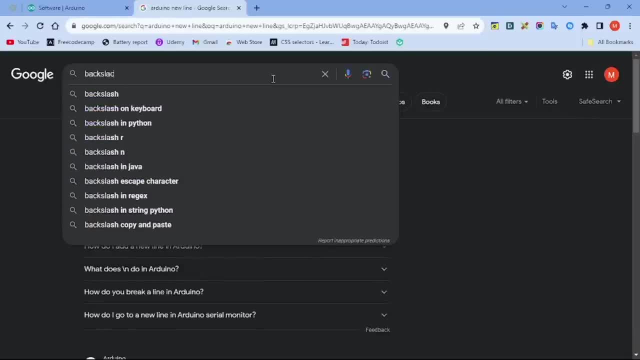 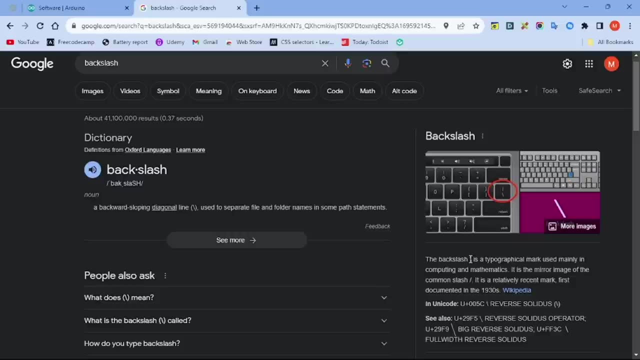 do is just say backslash, Say backslash. If you just find the backslash, all you have to do is copy it from here. There we go. You can do as well. copy it from here Again. you guys can see, right here, the backslash is right around here. 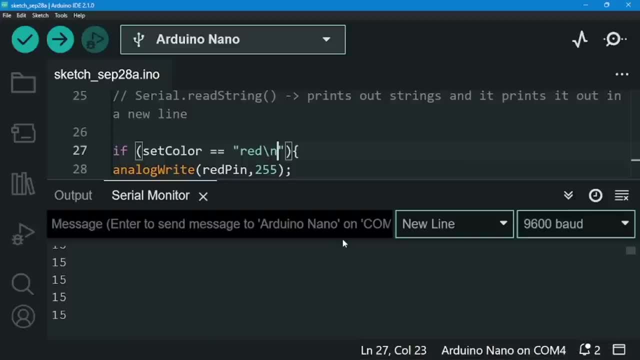 Okay. So even if you cannot find it, all you have to do is what? Copy this and paste it. Okay, Anyways. So you represent it with a backslash and an n. Okay N stands for what? For new line. 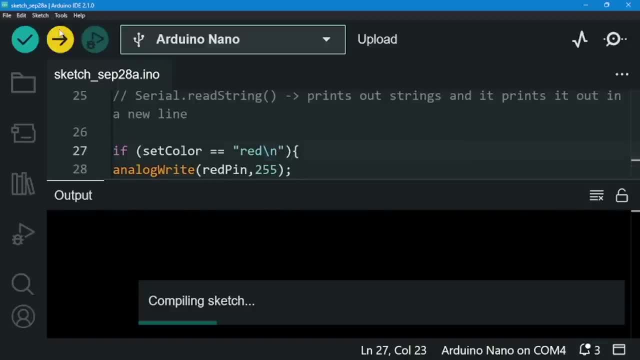 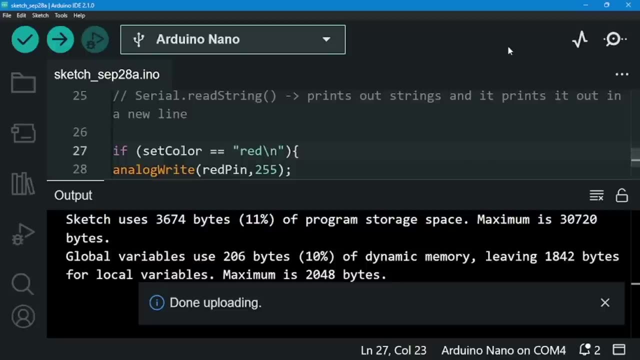 Okay, So let me go over here And let's try to upload it. Finally, let's try to upload it, And now I hope everything should be working, because we went through lots of errors in this section. So, okay, Let's go to our serial monitor right now. 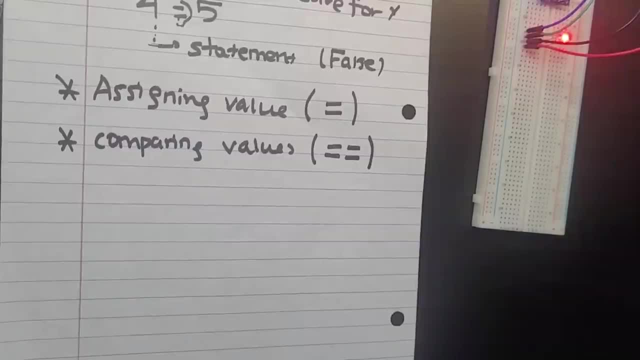 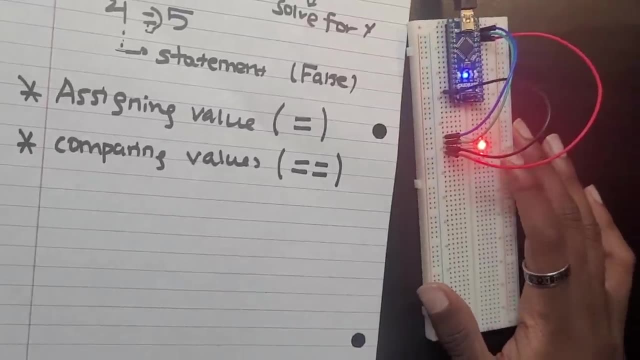 And let's see, And let's write down red, And finally it lights up what It finally lights up as what It finally lights up as red. There we go: It finally lights up as red. Okay, So that's one thing. 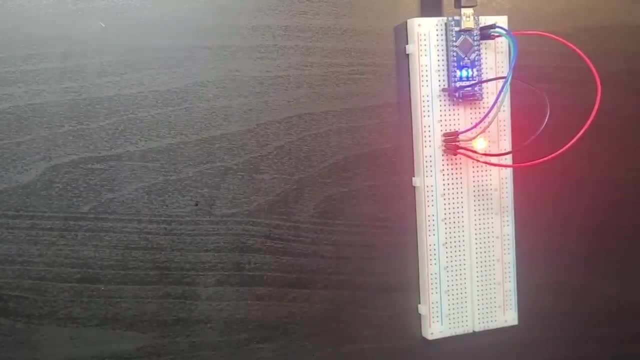 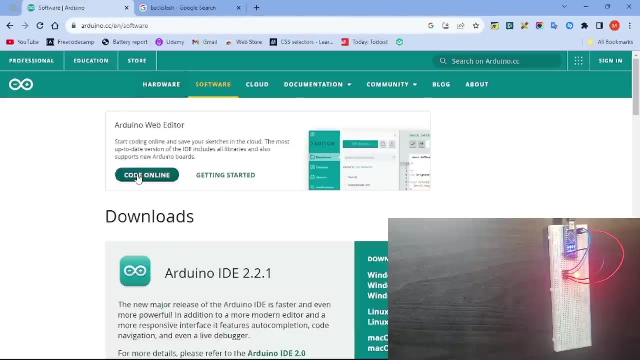 That's a very, very complicated thing, But let me explain to you guys why this is the case. Okay, So let me go over right here. So, for those of you who are using an Arduino version- older version, by the way, an older- 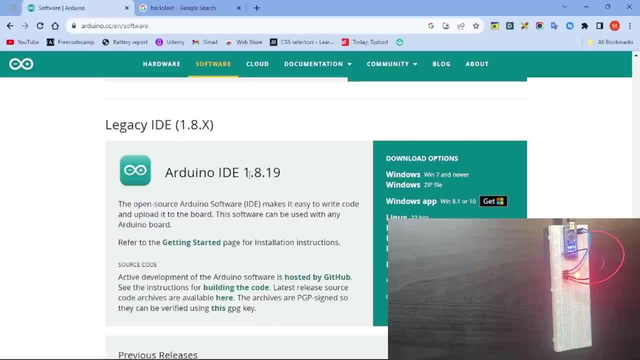 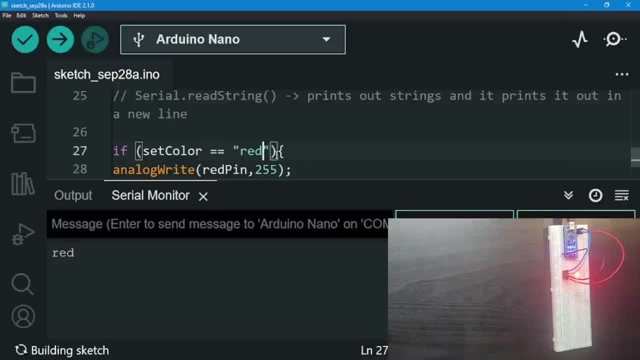 version, those legacy versions that are 1.8, you're not going to go through this error. It's going to work for you perfectly fine. Okay, So if we just say red set colors equals to red, it's going to perfectly work. 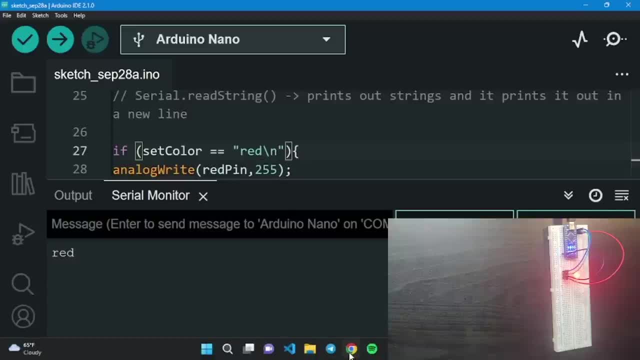 Okay, But after the ones that are using the newest Arduino. right now, at the current time of filming, I'm using an Arduino. Let me just go right here. The version is at the very top. I'm using 2.1.. There we go. 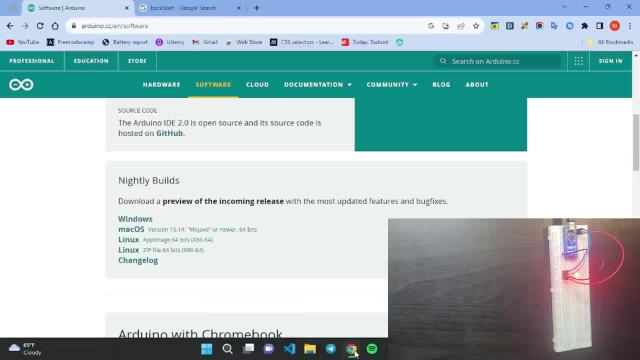 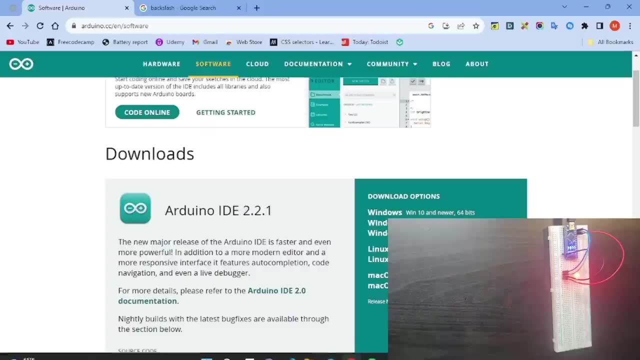 2.1.0.. So if you're using something around the two series right here, the Arduino, two point something series, Okay, What's going to happen is what you're going to have to use the new line. Okay, You're going to have to use the what. 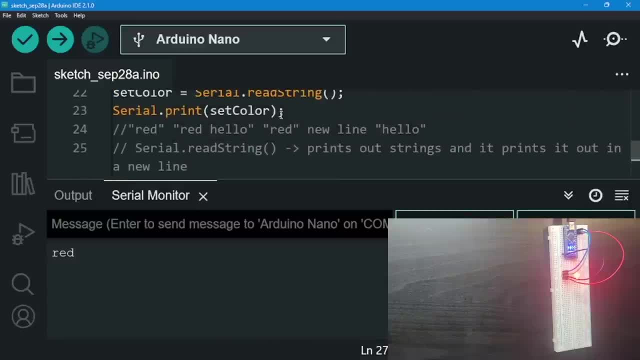 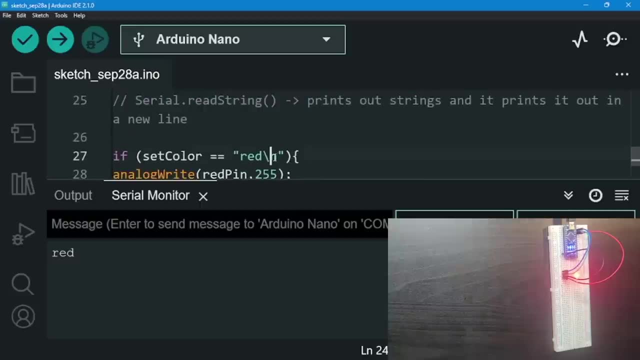 The new line character. Okay, So for those of you had again an older version, the legacy version, which is 1.8, you guys only need to do is what You guys only need to write it down as a normal string. 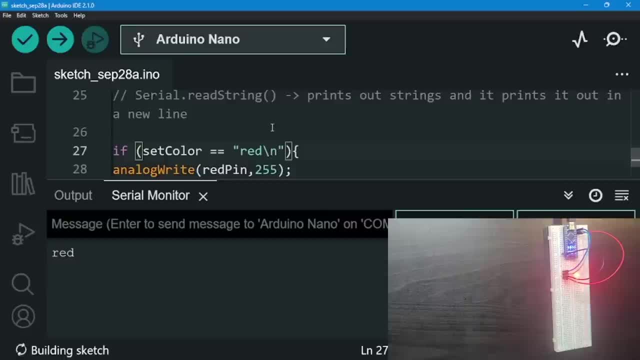 But for those of you, there is what, There's the addition of what, There's the addition of new line every time. So what does this mean? by the way, What other analogy we can use is actually a good example would be print serial dot print. 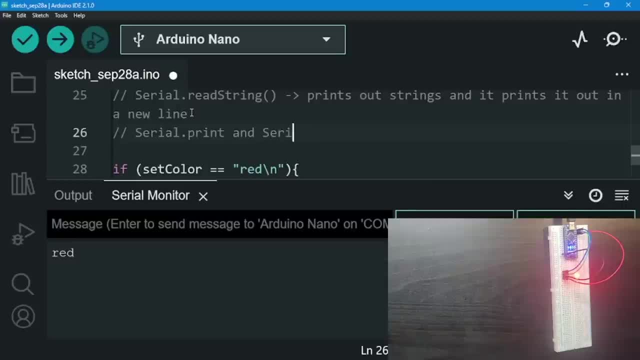 and serial dot. what Serial dot print ln? All right, Print ln. What did we do when we were using serial dot print? This basically means what It prints it out and it's next to each other. That's what happened When it comes to print ln. what it did was it just printed the serial first. 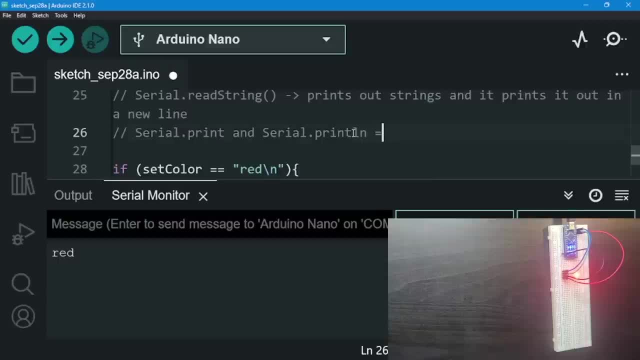 It was just a combination of what. It was a combination of, basically, serial, what Dot print And we added what. At the very end we added the character what, With a backslash right. here Again, backslashes are important, Not a forward slash. 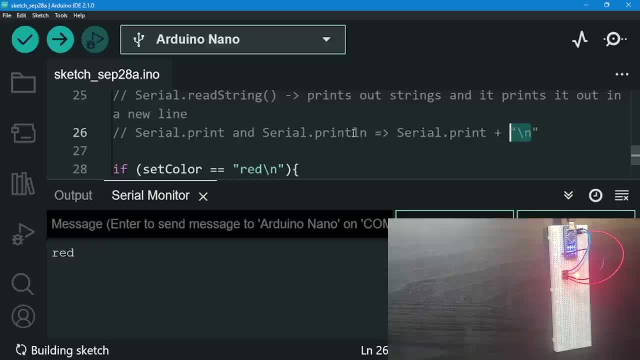 Backslash and with the what With the new line character. That's basically it. Serial print ln. was what Serial print Added with what With the what With the backslash and what Character, Basically meaning a, what A new line. 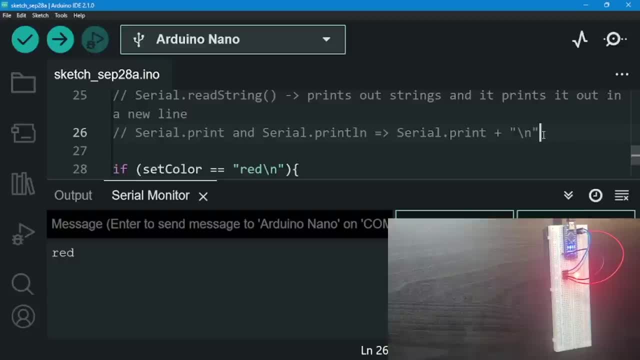 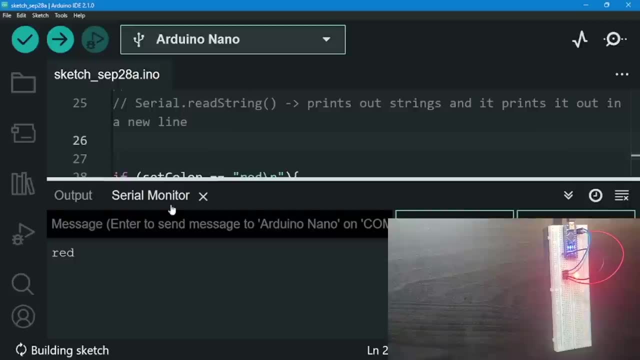 Okay, That's all I want you guys to keep in mind. All right, So right here, we just only added red, So let's add a few more colors. I think this is going to be the most exciting section of the course, because we went through. 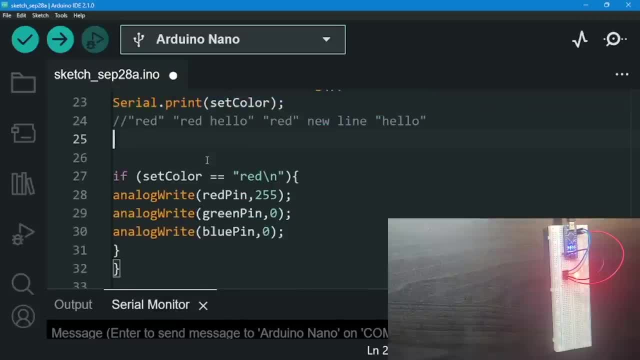 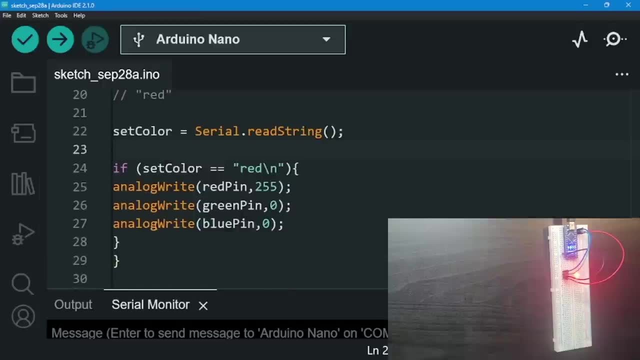 a lot of errors before even getting close to here. So let me just remove all these codes that are unnecessary. All right, there we go. Let's just improve our code right here. Okay, So what else can I use right here? What can I say? 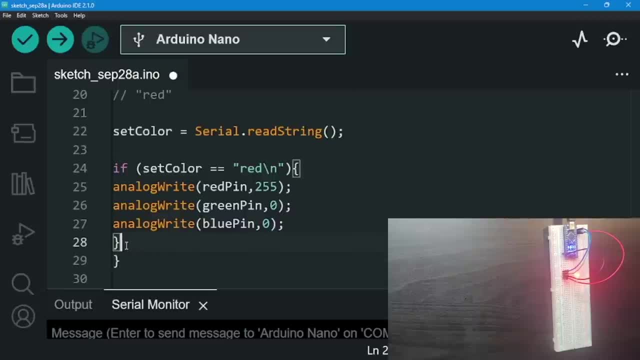 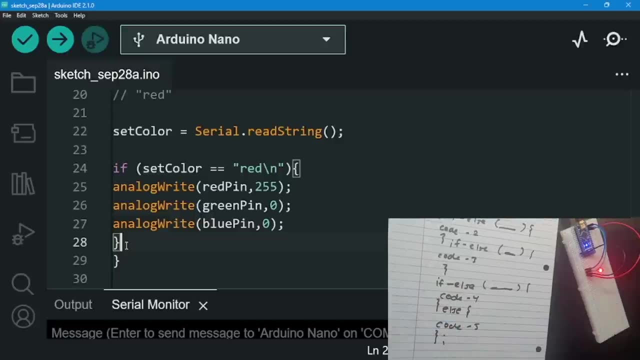 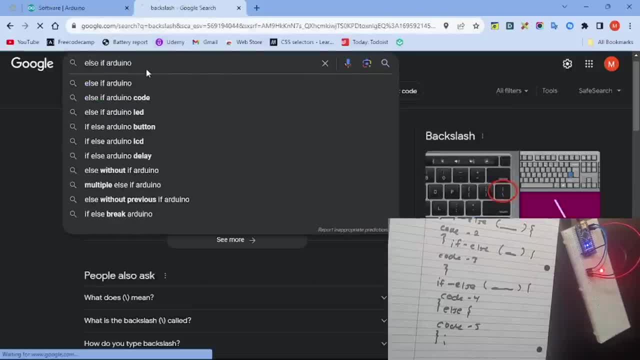 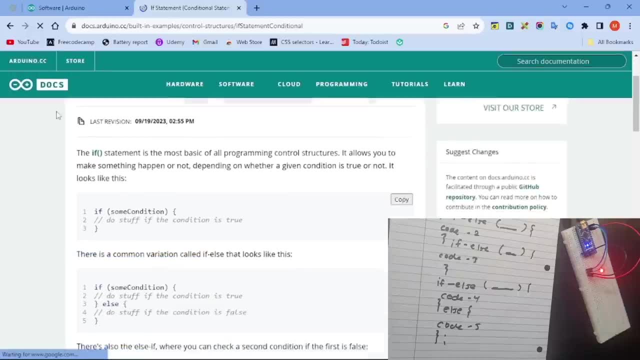 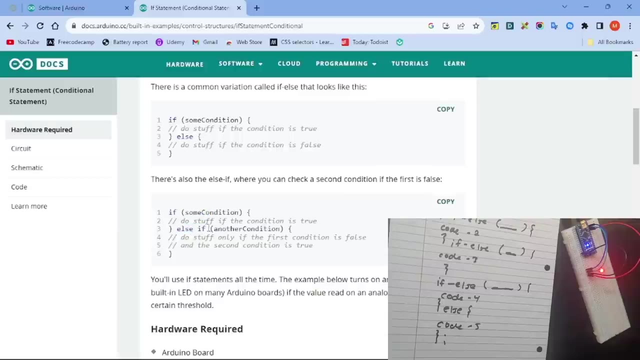 Say: else if Arduino? Let me just Let's go over to an Arduino again. You always have to what You always have to read documentation. There's if there's else and there's what else if. Okay, So the naming is different when it comes towards what type of language we're using, but it's. 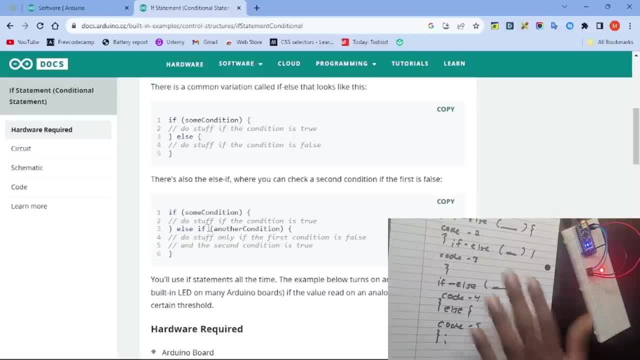 an if else, or you can call it else. if It's again preference, You can call it if else, or else if, But you have to write it down as else. if, when it comes to what To Arduino, There we go. We have to write it down as what. 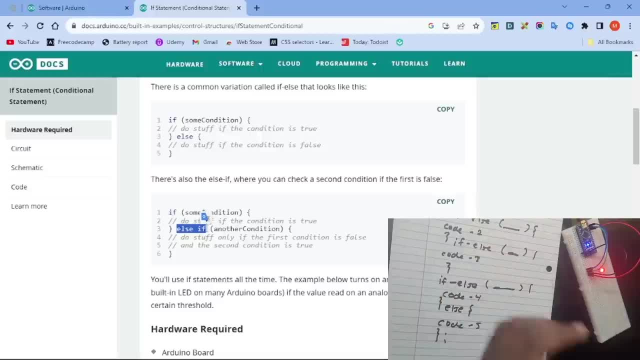 Else if I teach this as if else because I was using a different. I use a different language to code and it's written down as if else in another language. Okay, Another coding language, But right here we have to write it down as else. if 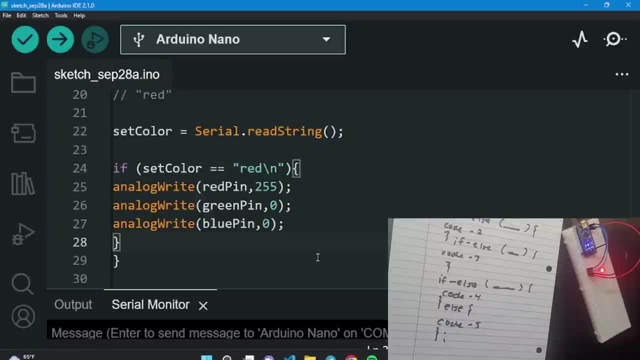 All right. So what I have to do is right here is say: okay, this is not red, What I want it to be is what it is. All right, I want it to what Let's use, let's set up. let's say, this time let's set up cyan actually. 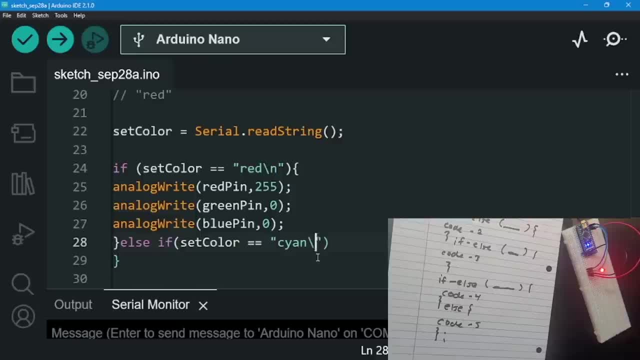 I want to set up cyan. I really want to set up cyan, Obviously, give it a new line right here And then, after giving a condition, obviously, what do I want to do Now? I want to do the analog right Red pin for cyan. 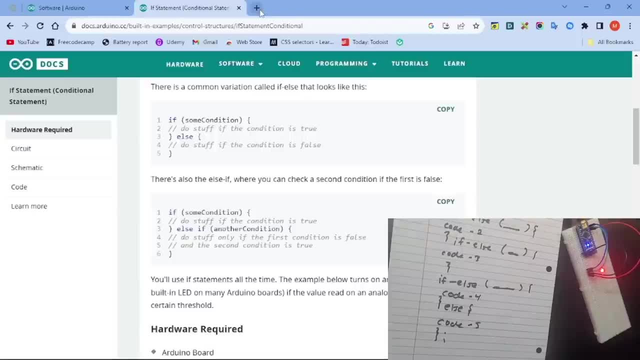 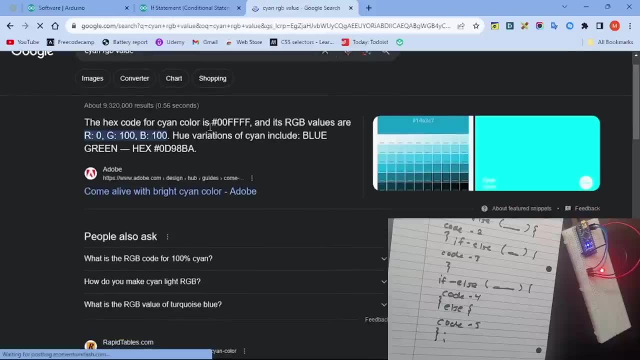 I don't know what it is. I have to first. I have to first what. Google it. So let me say cyan RGB value. The RGB value of cyan is what Red of zero and green of hundred and a blue of hundred? 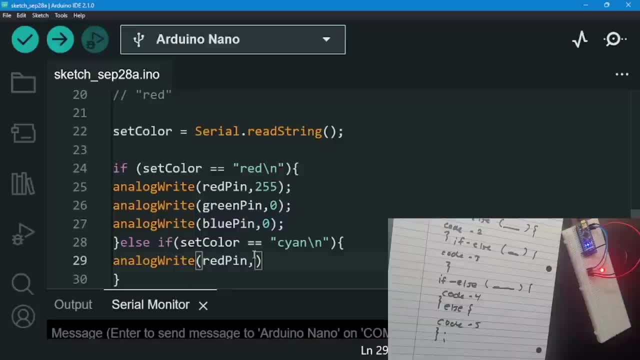 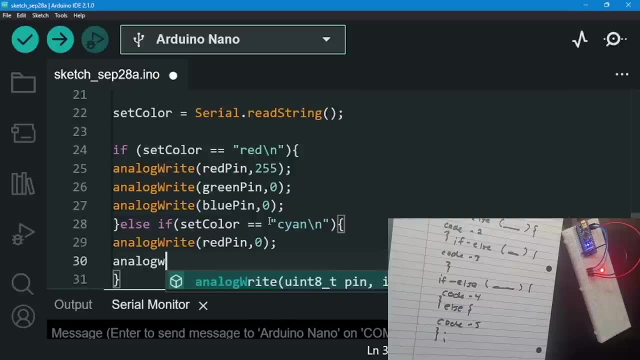 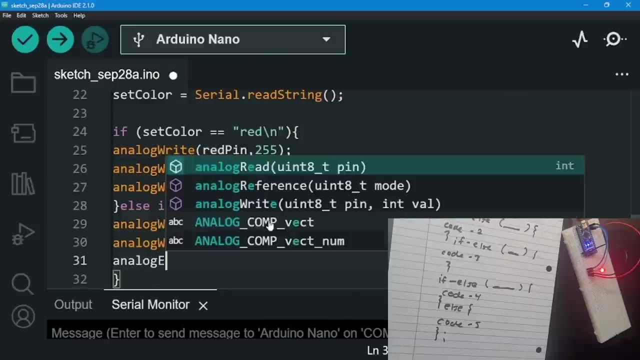 Okay, So let's just do that. So let me go right here. Red of what Zero? Green of what Hundred, We'll just go analog right. Green pin, Let's give it a hundred value, And then we'll analog right of what? 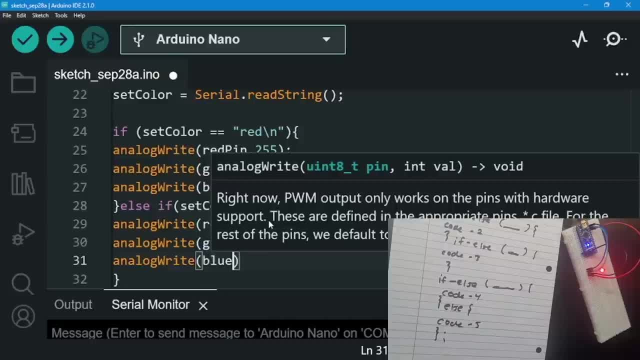 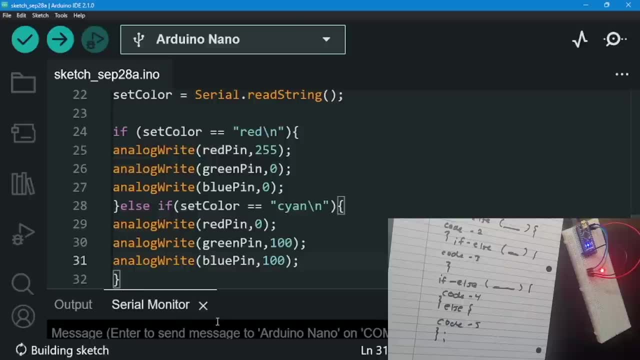 Green, sorry, red, blue, blue, of what Hundred right here And let's set it up. Okay, So I want to upload it. Let me just turn off my serial monitor right here And I think this is good, All right. 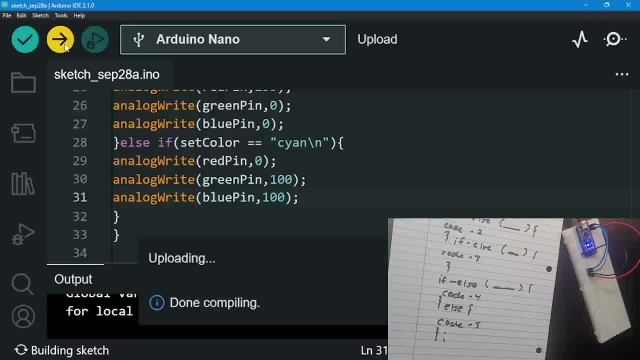 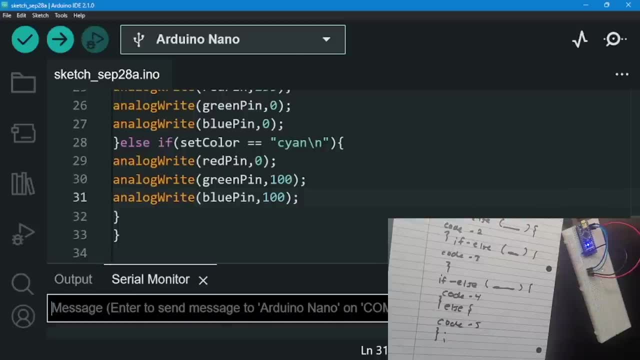 It's good, Let's go to our serial monitor right here. Okay, I'm going to upload it right now and should be working good, Let me just try to see right now. Let me just see red right now. There we go. 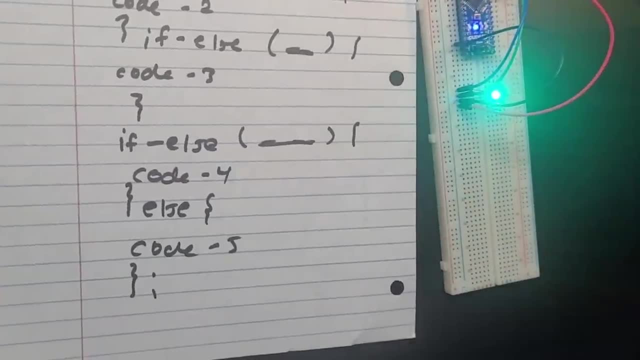 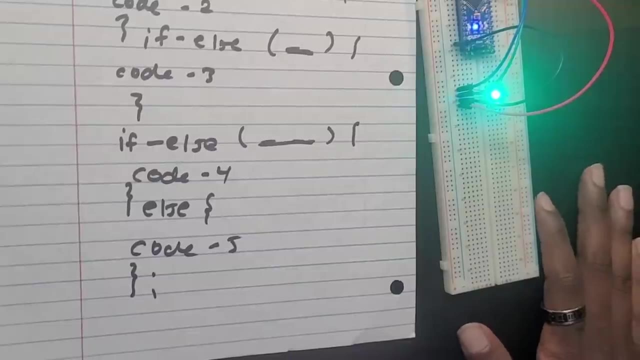 How about cyan? There we go. Changes to cyan. Hopefully you guys can see it. Let me just see if you can see it. Some of what Greenish type of blue Again, if you can see it Looks beautiful. Then you can add more colors too. 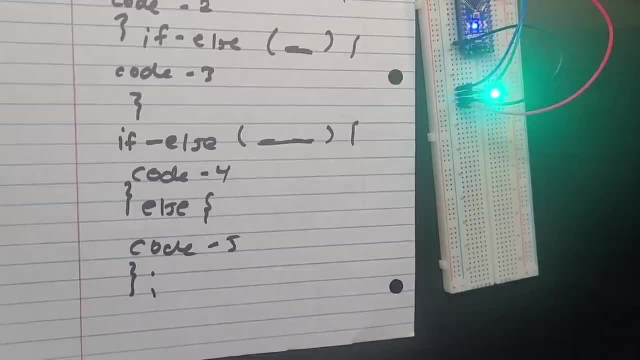 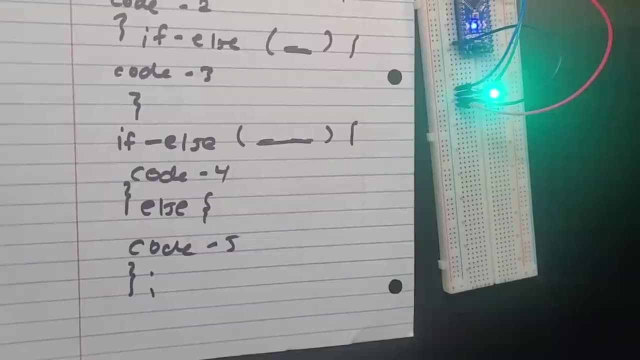 You can again add pink, You can add what Purple, It's up to you. again, Add your favorite colors. This is going to be a project: Add three or four, Four of your favorite colors and then fully create what I just did, right here. 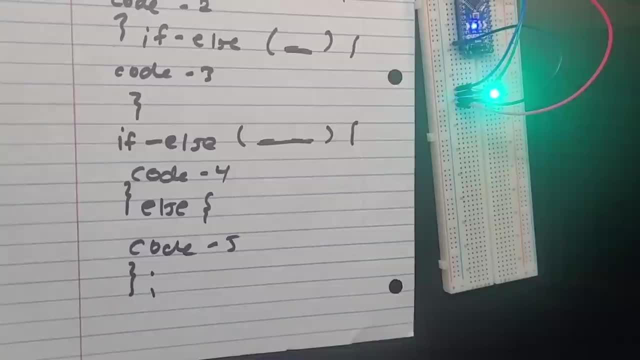 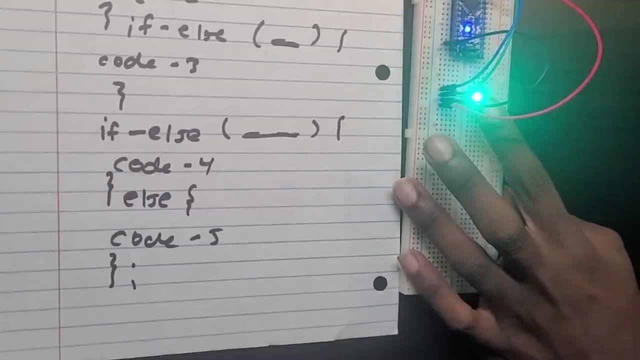 Okay, I just want you to do that. That's all you have to do, Okay. So, anyways, this was a bit of a longer section, a bit of a bigger project. We finished it, It was a success. So, anyways, see you in the next section. 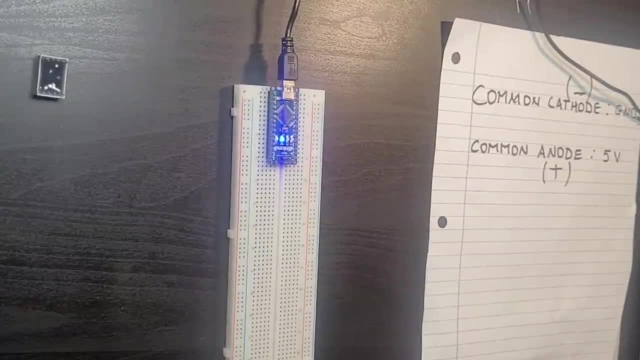 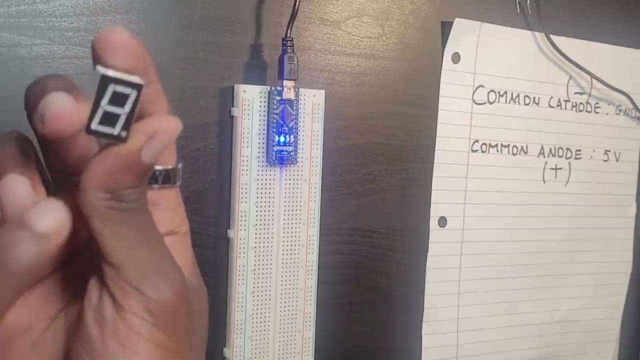 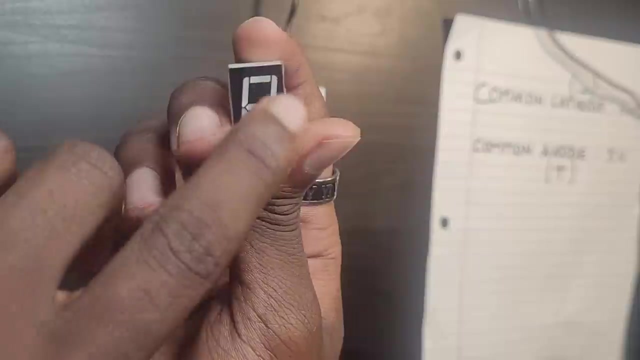 Okay, so let's go to the section. So right now, what we're going to be discussing about today is LED displays, So the seven segment: LED displays. So this is going to be our first time in this course working with some sort of display. 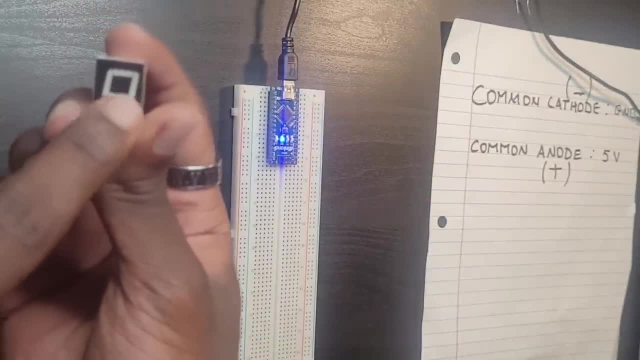 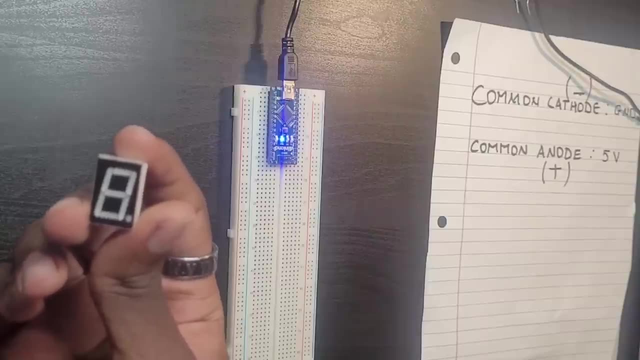 Okay. So this display- I think you're familiar with it, as in: we use it in digital watches- not only digital watches, but calculators- And even when it comes to, Let's say, we're going to a gas station to again fuel up our car. 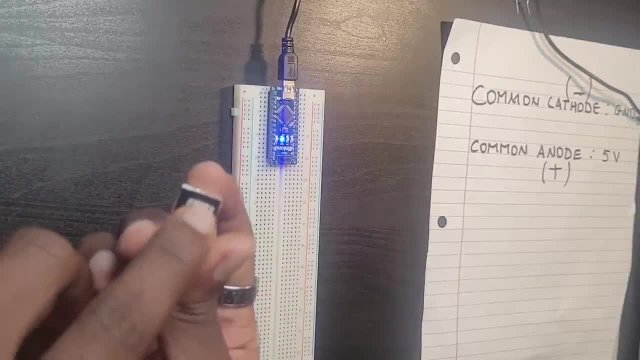 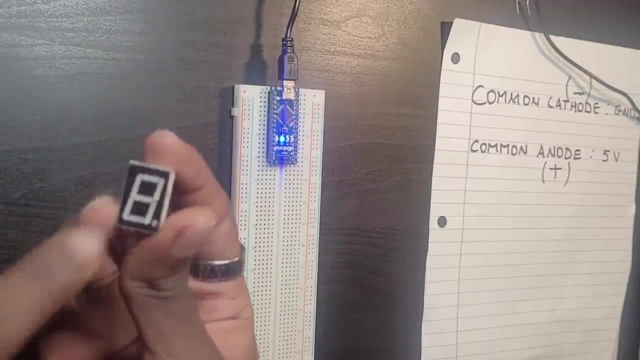 We can see what We can see: the price per gallon stated by these type of displays and even the total price being displayed on what? By using these type of displays. So we see them very, very lot often. So what are their use? 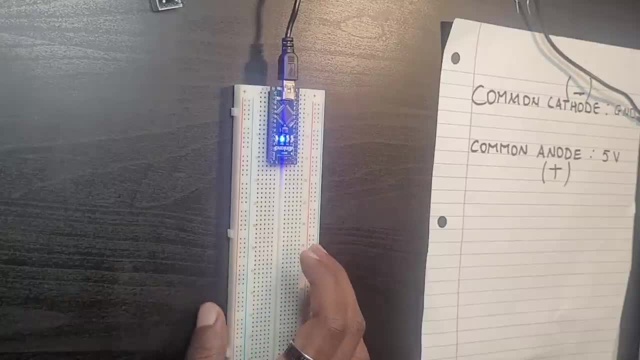 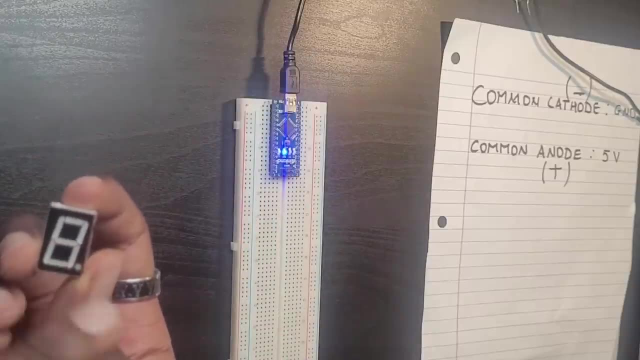 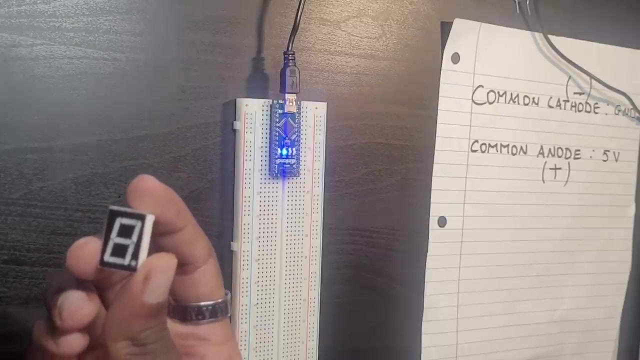 Their use is. we use them when we want to what, When we want to only get numbers or alphanumerals. These are capable of what? Only displaying alphanumerals, Alphanumerals and numbers. So, for example, we have LCD screen when it comes towards our laptops, our devices and 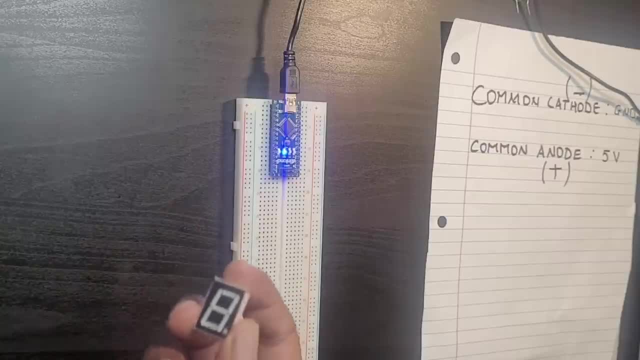 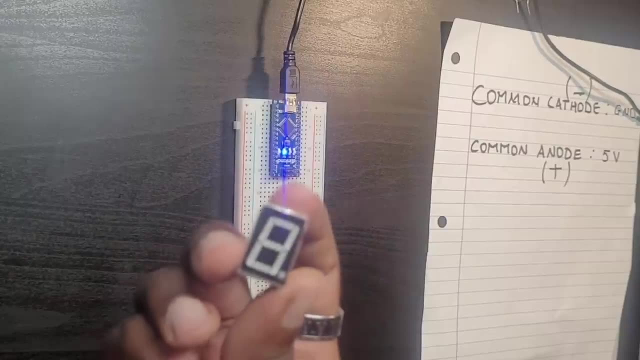 all that, They have a dedicated display. But what if you need a very cheap display that is supposed to only indicate number or sometimes letter? So in this case, the effective solution is going to be what? Having these cheap LED displays. Again, they are very, very little. 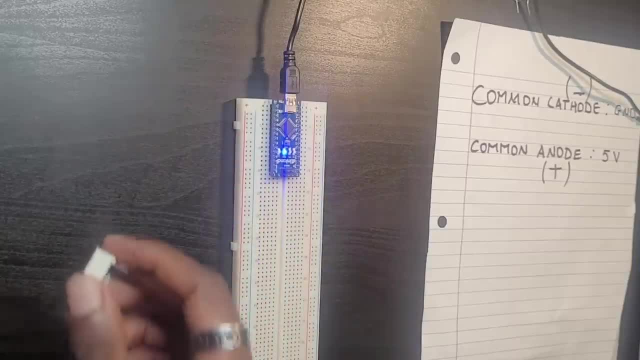 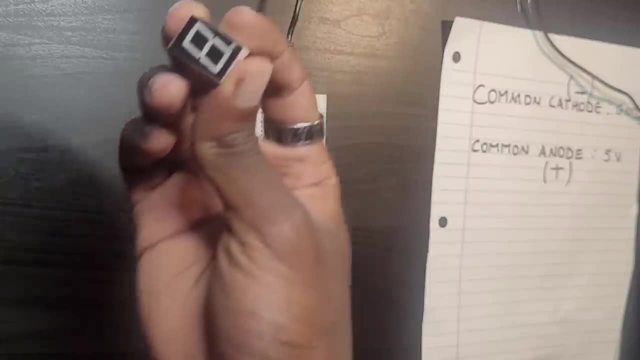 Not only that, too, but they're very, very cheap. Okay. So when we're using again, Okay, When we don't want these smart LCD displays again to again use them on devices that are unnecessary, when they're unnecessary, we use what. 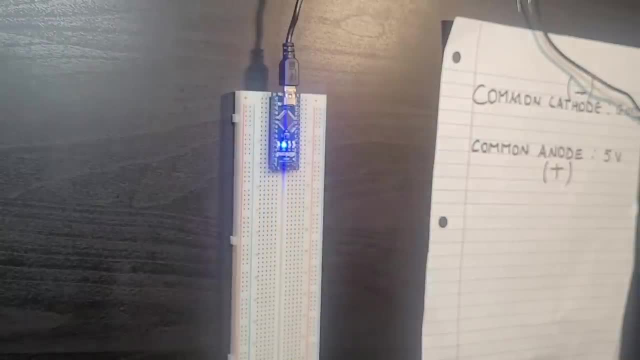 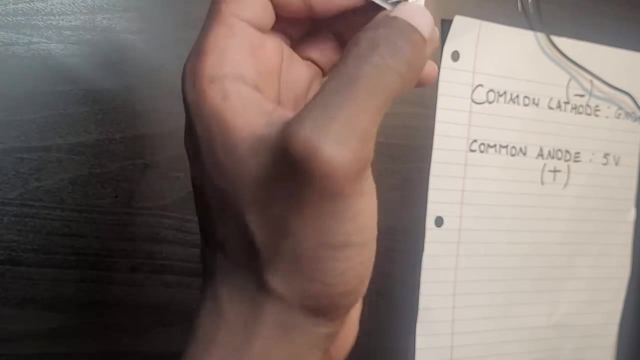 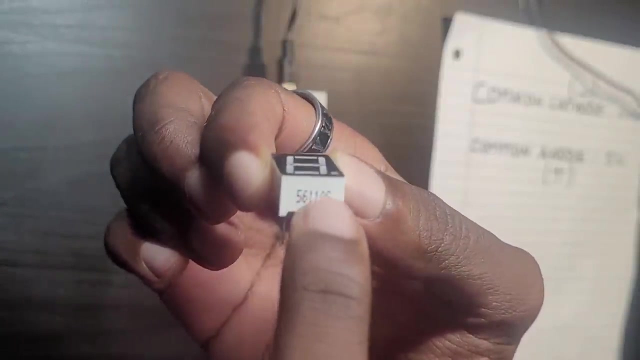 We use LED displays. So right here, we're going to be using it. So right here, one thing you need to understand is, when it comes to LED displays, right here, when you go over, there is a specific number associated with your specific what. 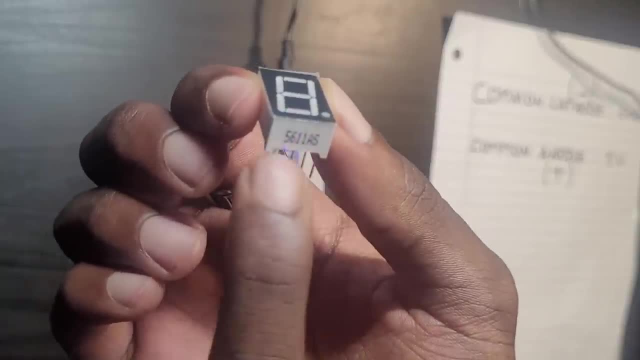 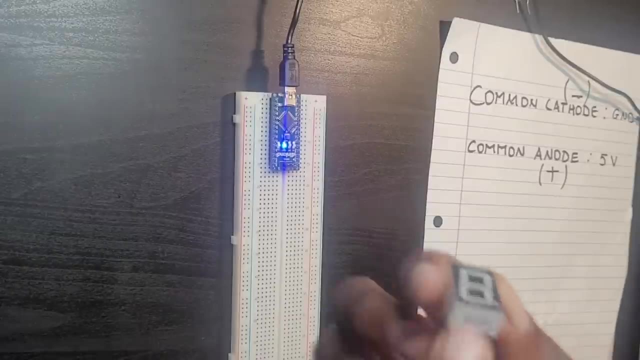 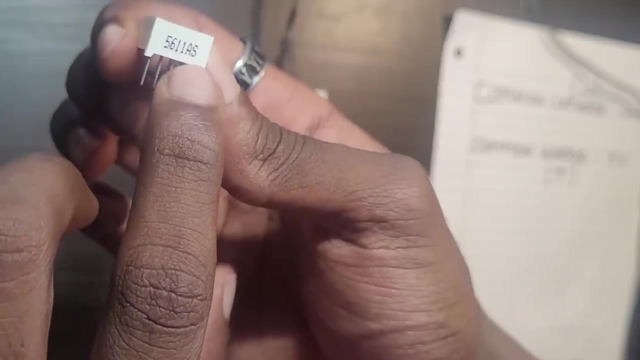 With your specific manufacturer, Basically the one the type of what? the type of LED display: seven segment LED display. So, before doing anything, what you first must do is literally go here, Google the name right here. say: right now, mine is 5611AS. 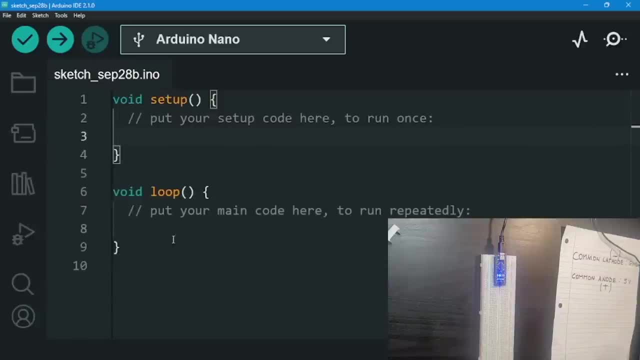 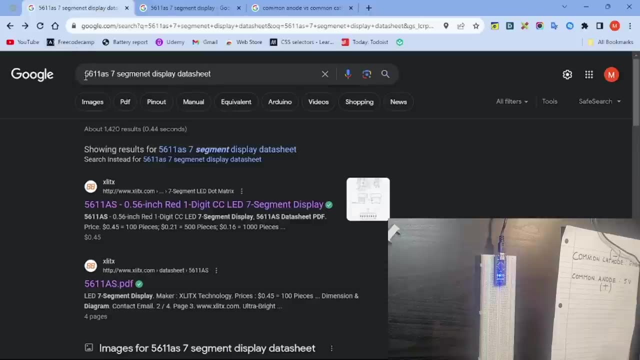 Okay, You have to go to my. let me just go over to my screen right now. So, before running anything, first thing we need to do is Google 5611AS. This is again my number. you Google your own number. 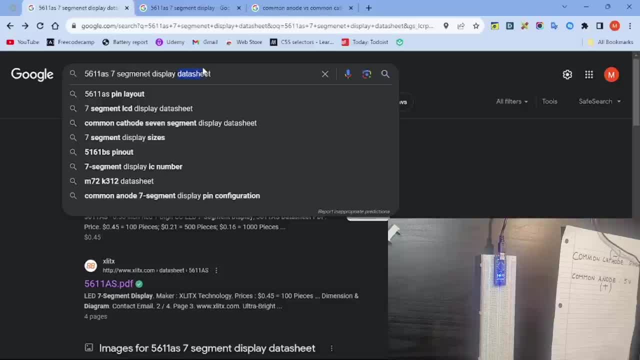 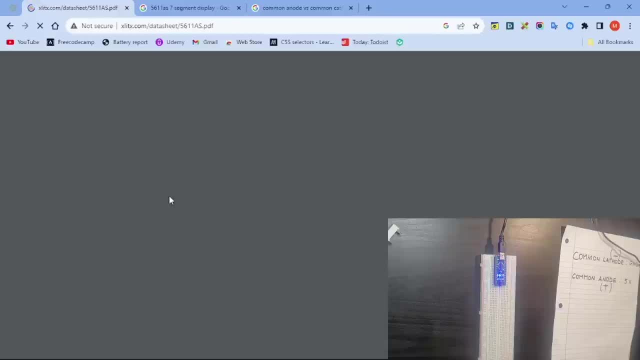 Yeah, I just want to say now it's 5611 Gorilla板 on 777-segment display D2C. okay, Once you do that, go towards the link that has PDF, Or you can go over and get the website check it for yourself. 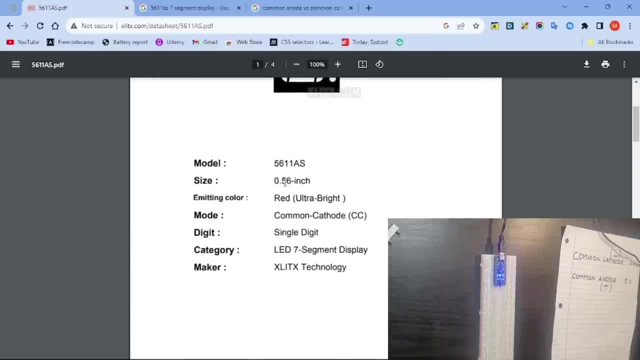 Okay, So I'm right here. And one of the things you can see what the size. you can see the emitting color. it's going to be red, Some of them are blue, But most of them are red, and it has a comat cathode. 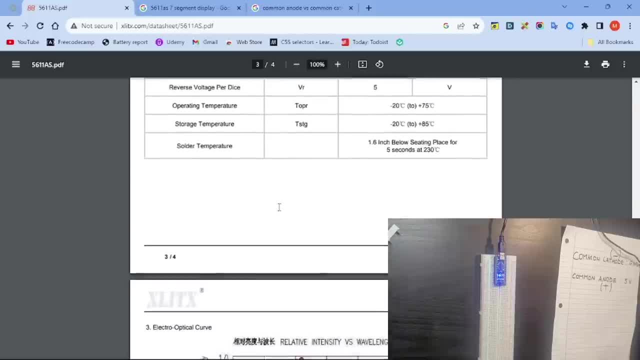 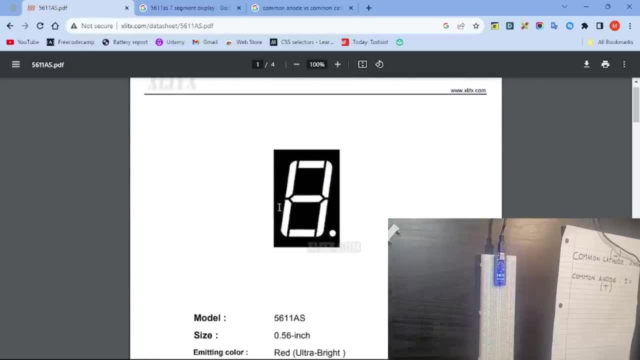 I'm going to get to this And it's obviously a single digit And it gives me all the information I need for the display. Okay, on what on this? what on this led display? the seven segment led display. okay, so right here you might be wondering what it. why? why do we call it a seven segment led display? so let me just go. 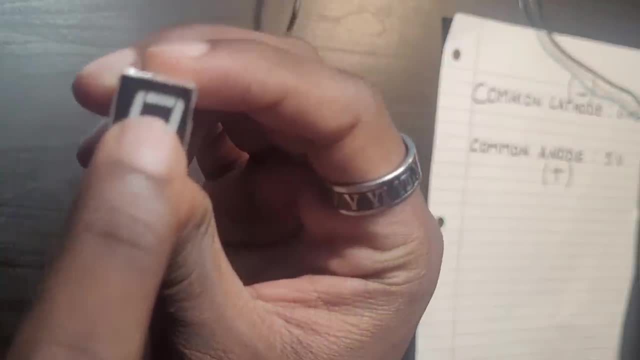 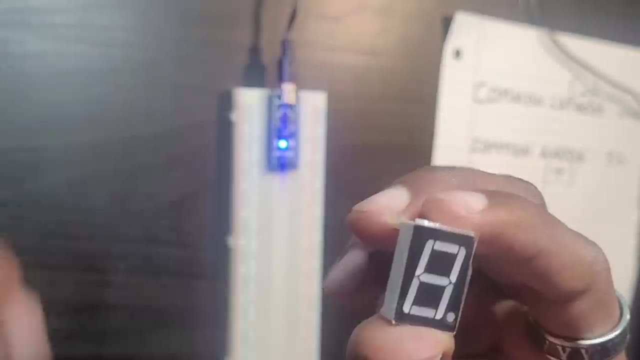 over right here and when you just read this, when you just look at the seven components right here, let me just focus on the l seven segment led display. when you look at this, when you count this, let me just actually use a pointer, get my sharpie right here. when you look at this. 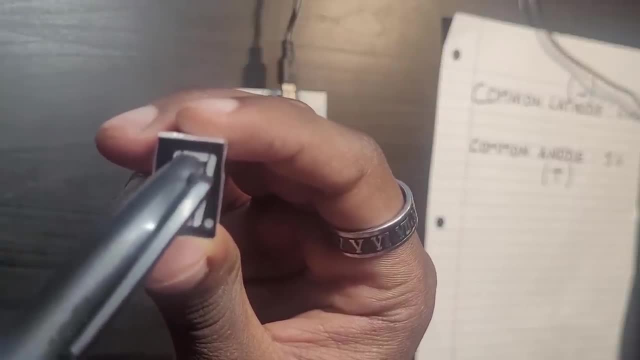 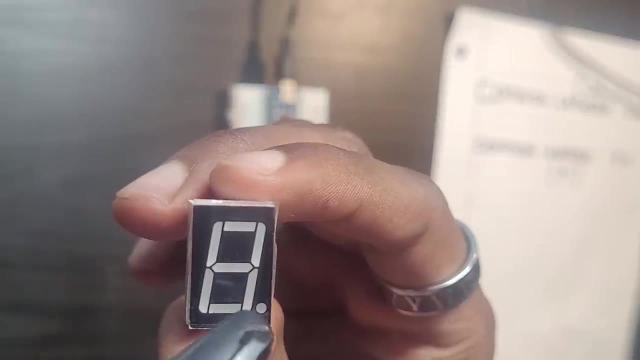 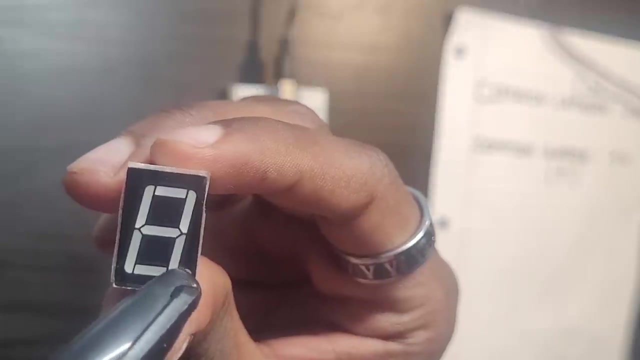 when you count this, it has seven segments counted, because there's one, two, three, four- let me just focus my again my camera on the led display- five, six, seven- there are seven, okay- and also has a decimal point. my one has a decimal point. yours might not have a decimal point included, but most 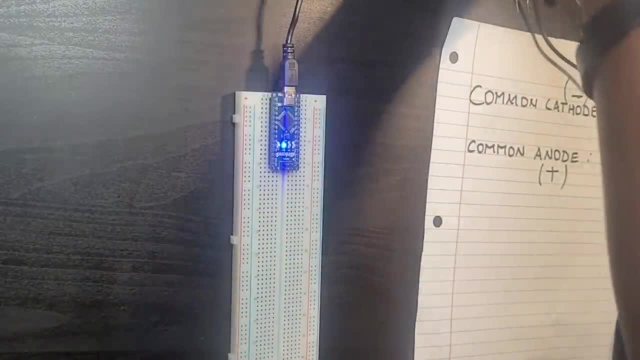 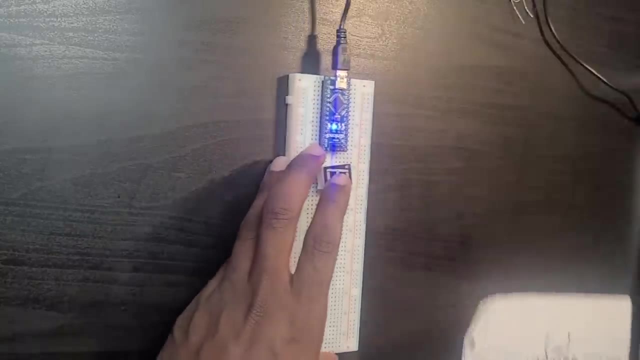 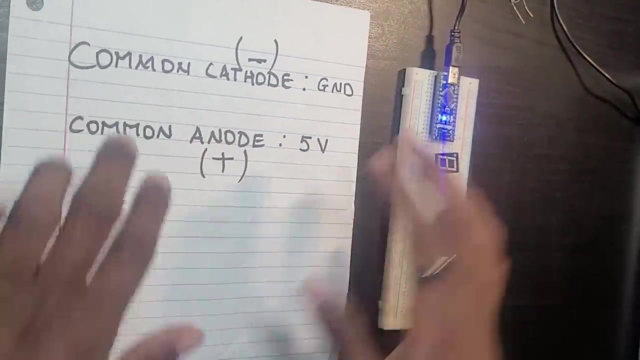 of them do, okay. so it's going to vary, as i said, from kit to kit. so again, know your number and read your sheet, okay. so before moving forward, i just want to declare something called common capote and common anode. so they come in two. again, they might seem the same. as i said, looks can be very deceptive. they. 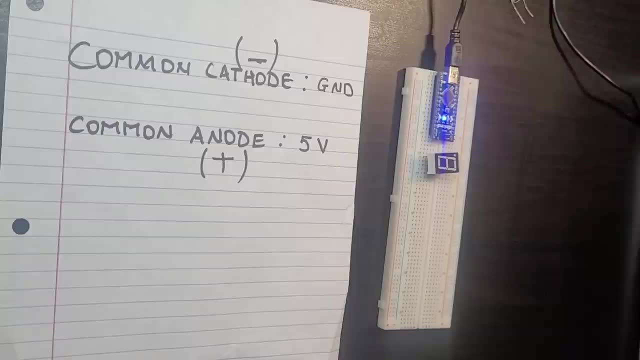 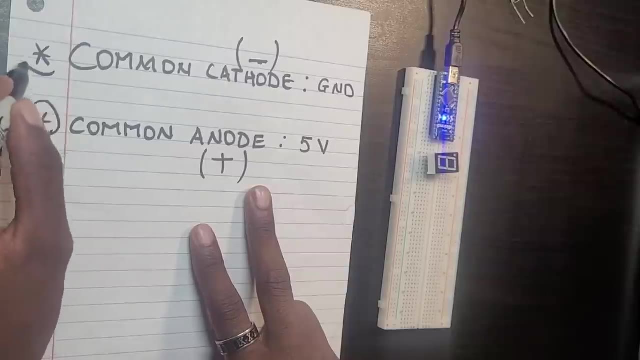 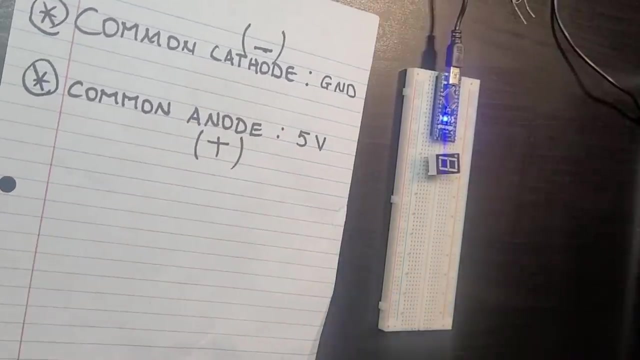 seem exactly the same, but they function again entirely differently. okay, so there are going to be two types of what led seven segment displays. so these are going to be common capodes and then common anodes. okay, so right here, as again, let me just go to my documentation, to my screen. when i do that, it says that it's a what? 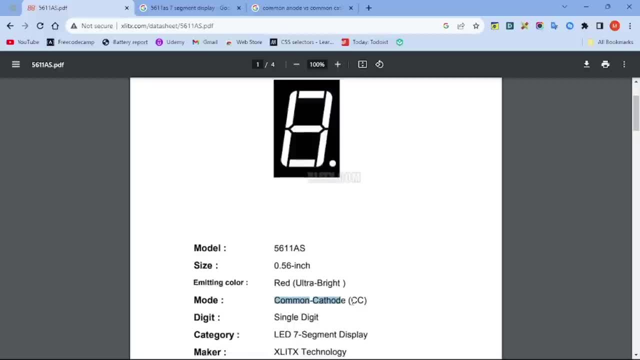 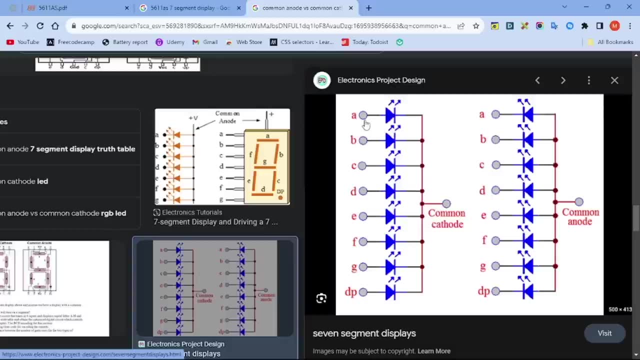 it's a common cathode, mine is a common cathode, so what does this mean? so let me go right here and try to explain it for you guys with this image, okay. a common cathode means is that there are different, as you can see, all the segments. the seven segments are right here. there are seven. 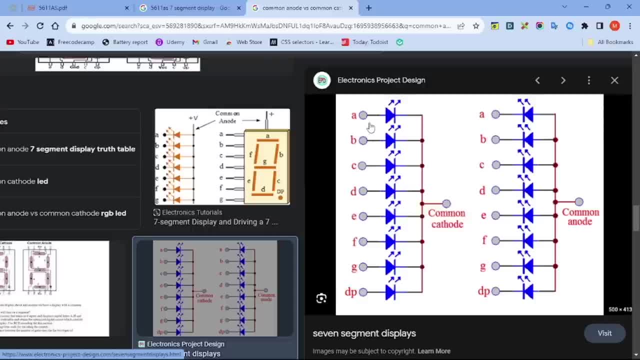 segments and then the decimal point right here, and what basically happens is what. they are connected to what? to a single common cathode. okay, they're connected to a single- what? cathode. so you can see they're individually right here. they have their own individual pins, as you can see. let me just go. 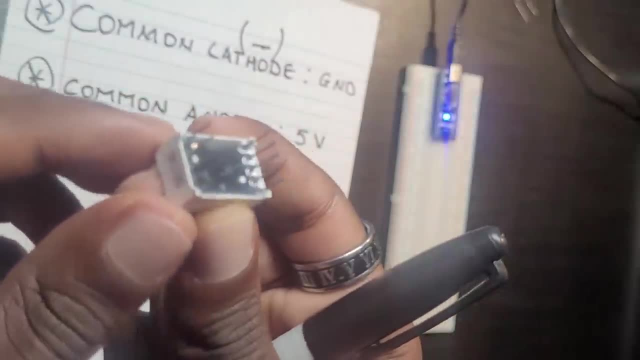 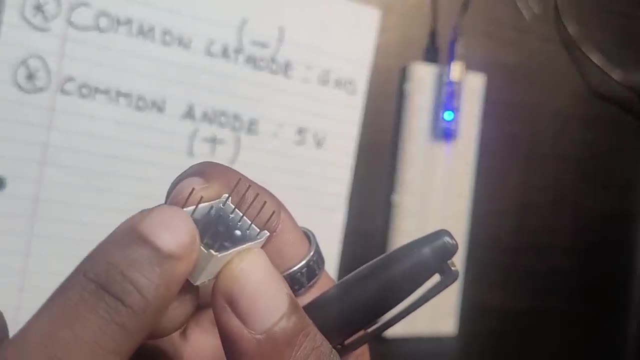 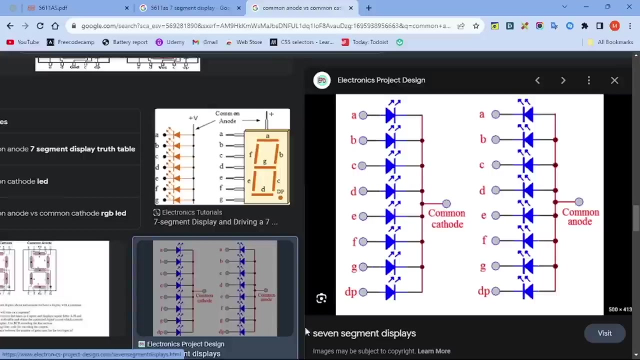 over to. let's go right here and show you on my camera. they have their own what? just focus on the? there we go. they have their own pins, as you can see right here. they have their own pins. okay, and then what happens is inside. they're connected to what, they're connected to a common. 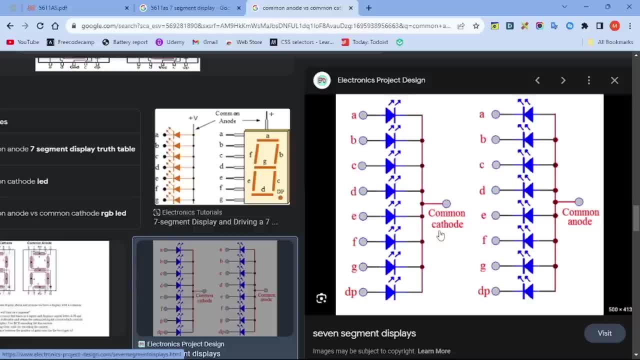 that's why they're called what common cathode. seven segment led displays: okay, when it comes to common animals, exactly almost exactly the same thing. okay, it's exactly the same thing. what happens is what it's connected to a, what that's connected to a common anode. okay, this time you. 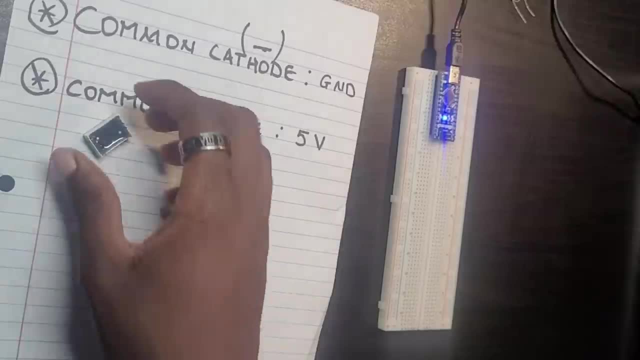 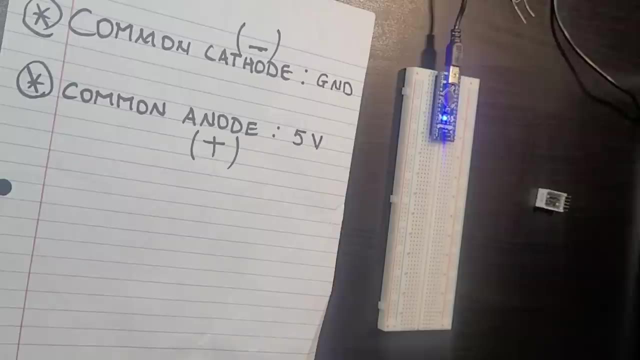 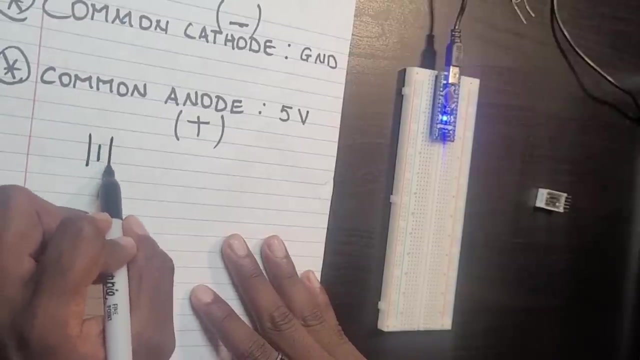 might not know what anode and cathode means, but cathode basically means negatively charged, anode means what positively charged. so to actually give you guys a meaningful sentence, what i'm going to do is draw a simple circuit, as we usually do. let me just do that. the longer side is the positive as 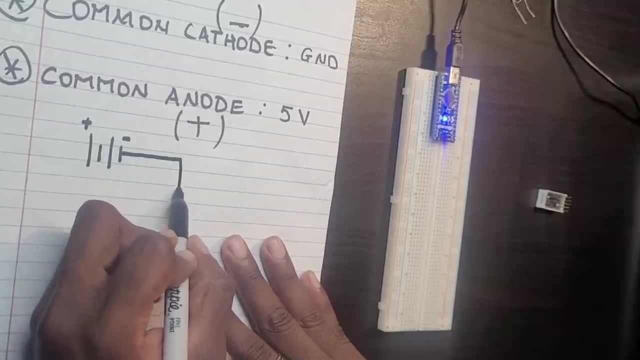 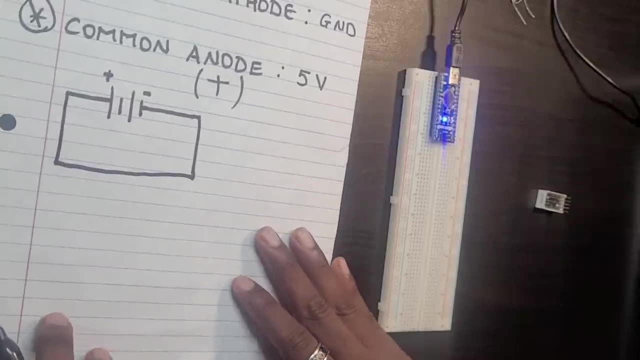 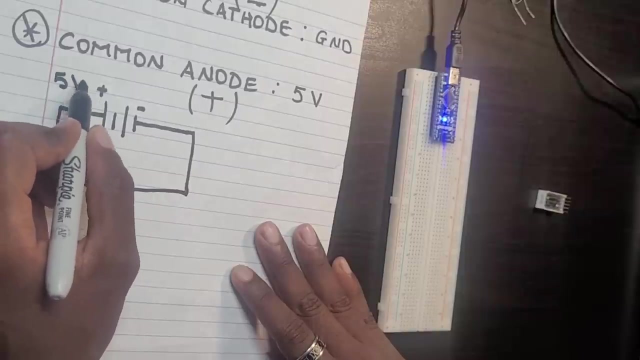 we know the shortest side is the negative and let me just throw that. okay, then, once i'm done drawing it, there's a positive side and there's the negative side. the positive side is what the five volt keep attention and the negative side is what negative side is where the g and d. 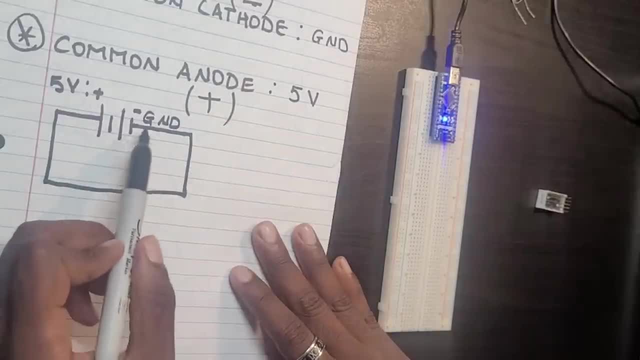 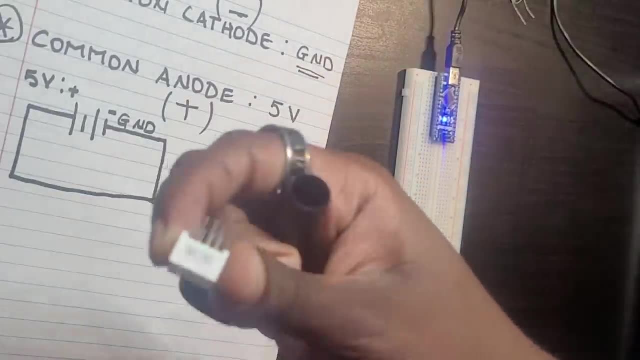 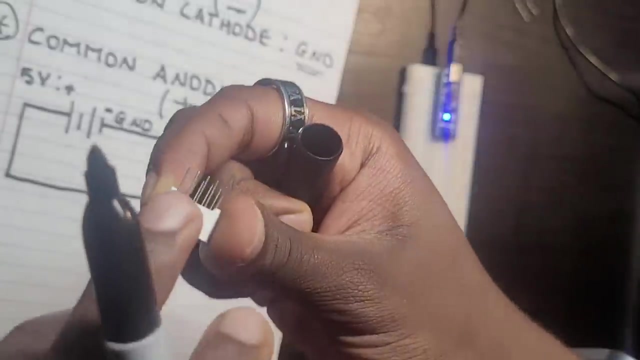 okay. so when we say we have a common cathode, what do we mean? we have a common g and d pin, okay. so for example, my case, it's a common cathode. i'm gonna have what i'm gonna need- only one gnd. because why? they have it all in common, so it's connected together. so again, they're connected. 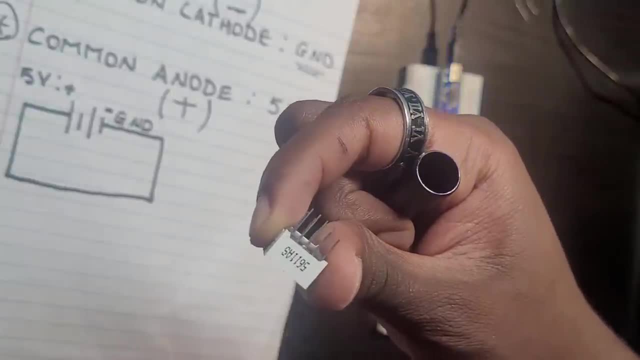 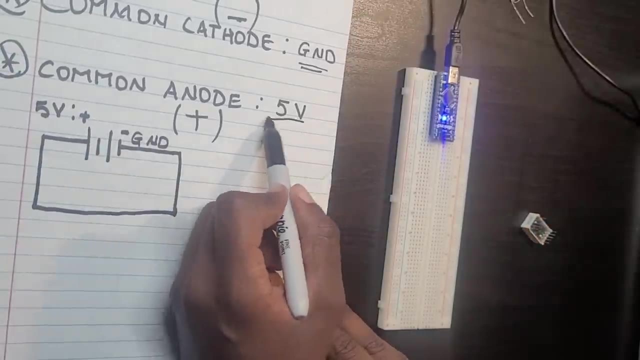 together at the very end and they have what one common, what's one common gnd pin? when it comes to the anode, it's gonna have what one connected five volt pin. okay, So I'm going to try to go over both of them: both common anode and both common cathode. 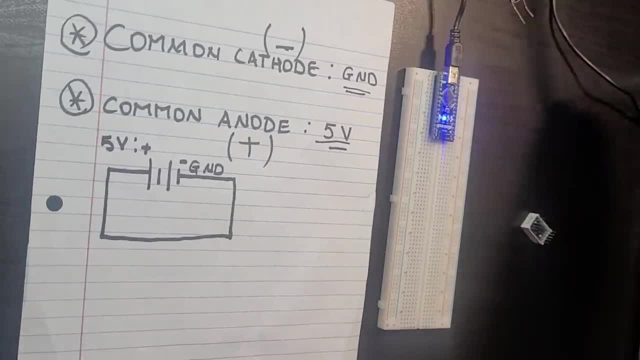 So you don't have to go through any other videos, You can just follow along this course. Okay, so let's get started. So let me just bring this right here. Let me just put it, And what I'm going to need you to Google is right here. 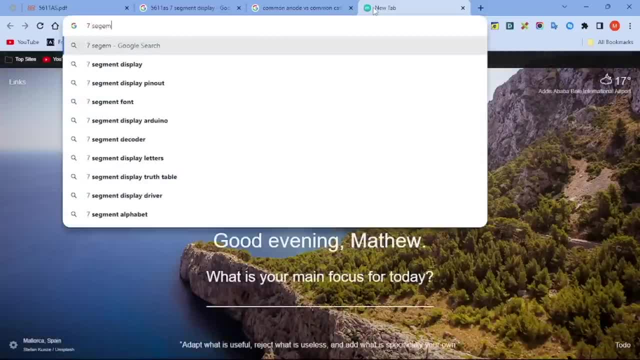 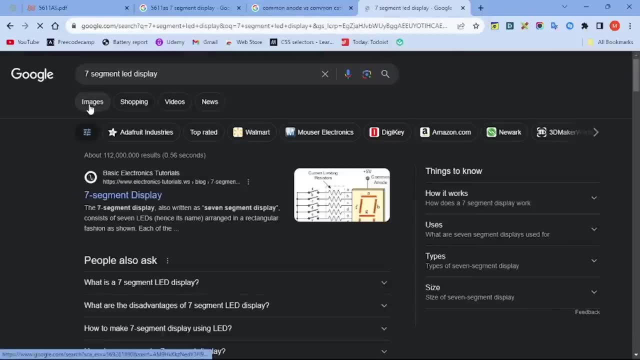 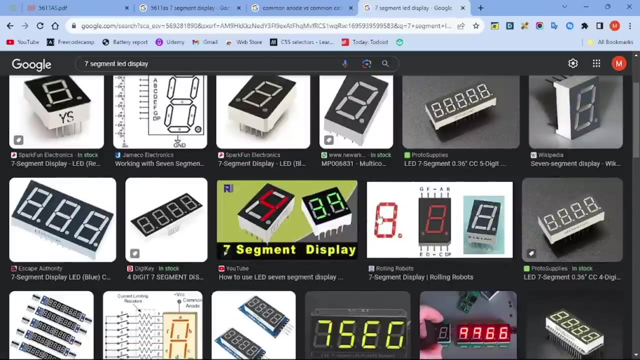 Go to seven segment LED display. Write it down: Seven segment LED display Right here. Once you do that, go to your Google images. Okay, And they show you the equivalent, what The equivalent pin. So let me just go over to this one. 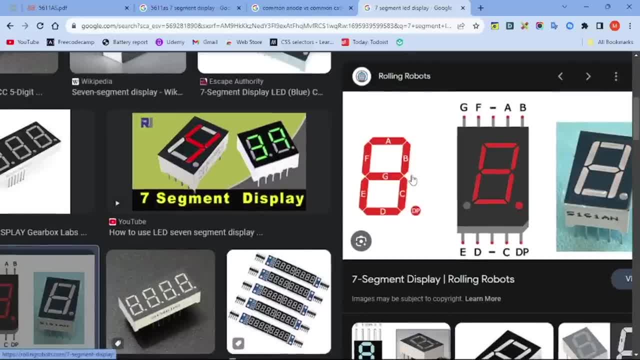 This one looks better. This one provides a more detailed image. There we go. So what can you see? right here It says G, F, A, B, basically indicating which segment it's going to. it's going to what It's going to light up. 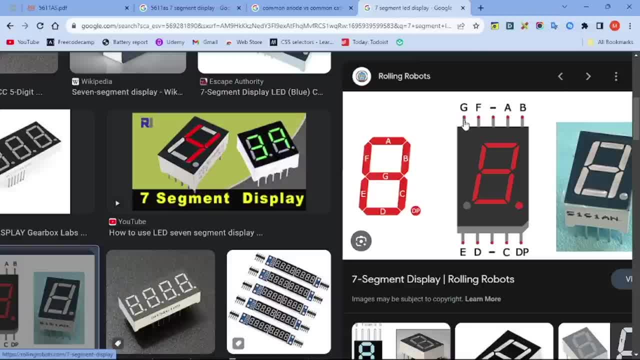 Okay, So G indicates what This one, So the first one that is at the very, very left, right here at the very, very left, is what The very, very left is, what It's G, Then the next one is F and the ones that are marked with again an underscore, a hyphen, 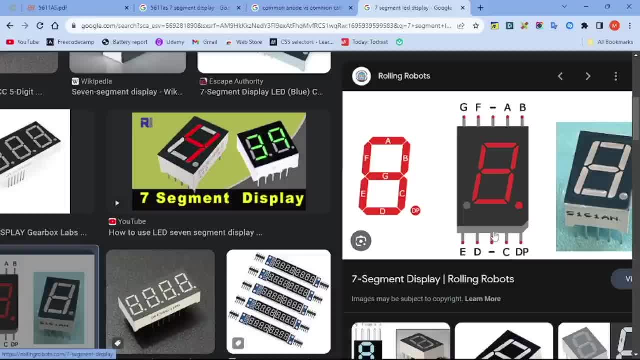 You can see, right here are the common grounds. Okay, They're the ones that are going to be what Those are going to be: GND if it's a common cathode and five volt if it's a common anode. Okay, I just want you to keep that in mind. 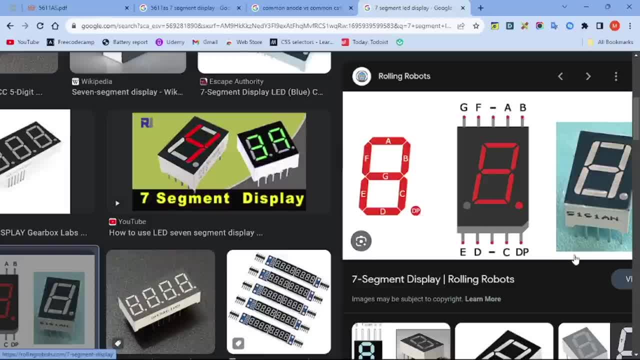 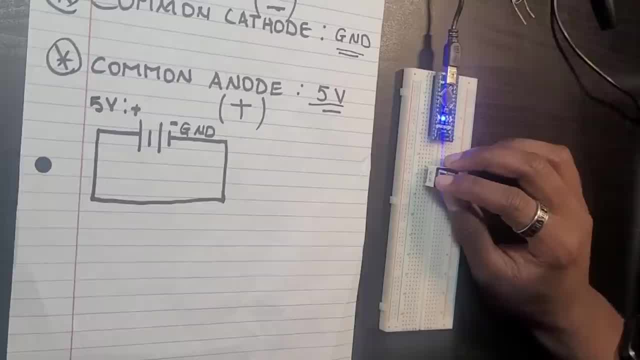 And A and B, and there's ED, C and also DP right here, Okay. So with that in mind, let me just try to light up my common cathode LED. Let me just do that. Let me just bring my LED right here. 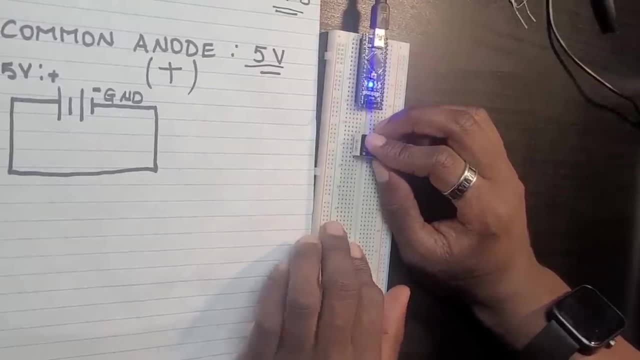 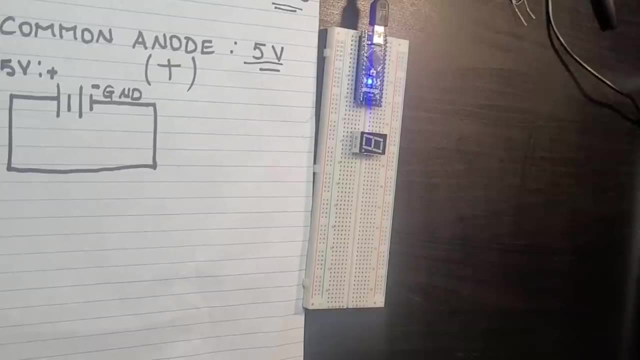 Okay, Let me just bring my LED right here. What do I need? I need a resistance right here. By the way, it's recommended that you use 500 to 1000 ohms of resistance. Okay, So 500 to 1000 ohms of resistance. 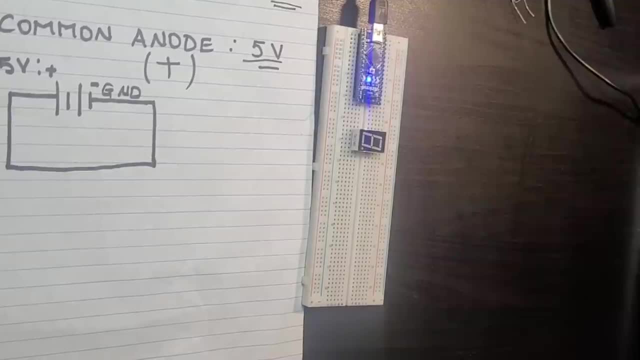 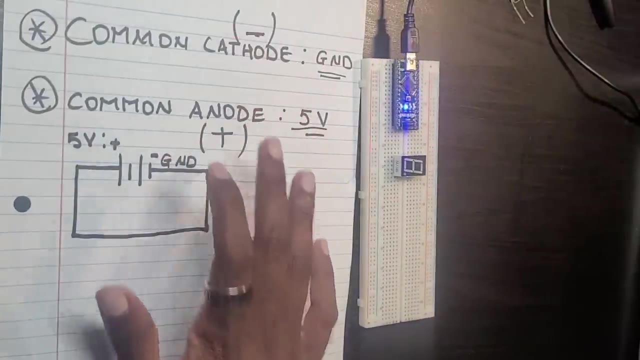 The resistance is going to be applied to who? The resistance is going to be applied to every individual pin? Okay, Except for the. what For the common anode or for the common cathode? Okay, Except for the common cathode and common anode, we're not going to apply the, as I said again. 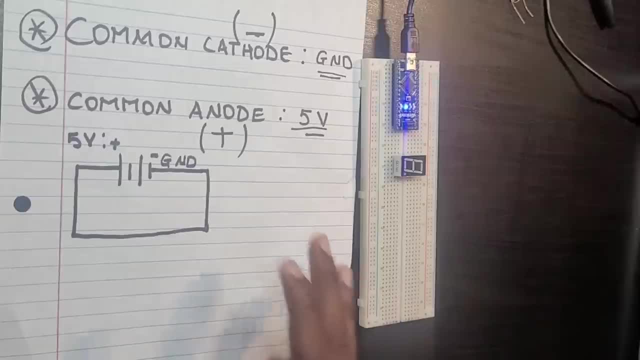 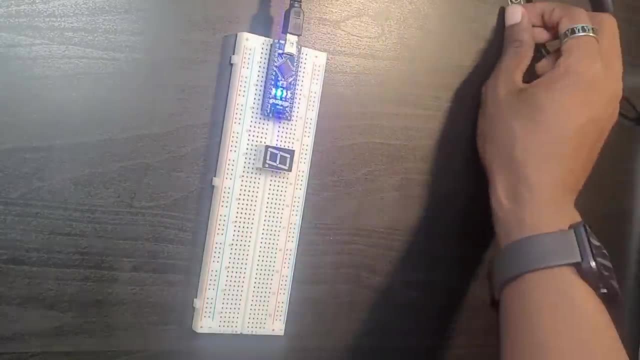 we're not going to apply the resistance, but where we're going to apply it is we're going to be applying it to every individual watt segment. Okay, Let's just keep that in mind, Okay, So let me just do that and bring this. 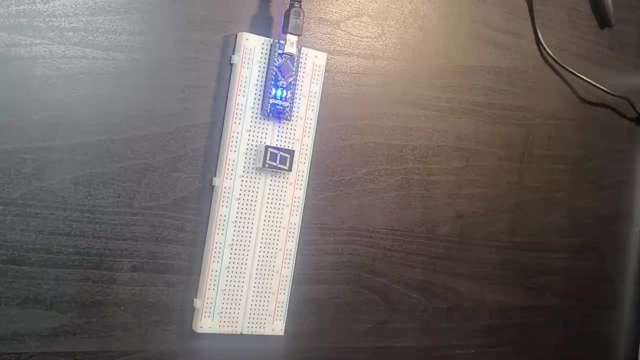 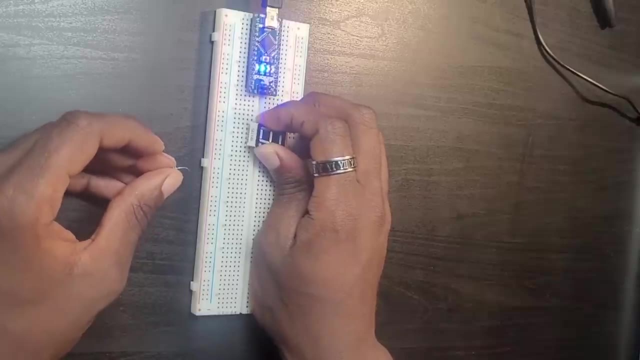 Oh, just threw a resistor. I'll try to find it later, Anyways, So right here, when I go to the screen again, it's going to be my guide. Okay, The G is located at the very, very what. 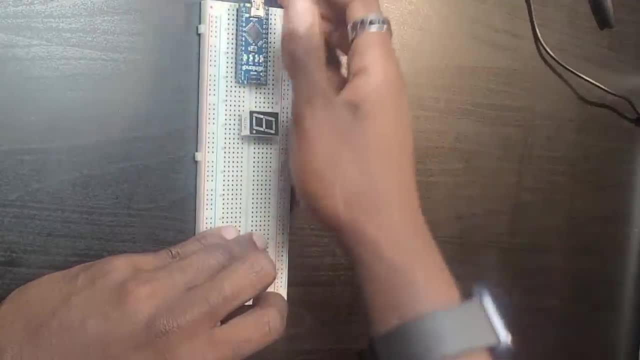 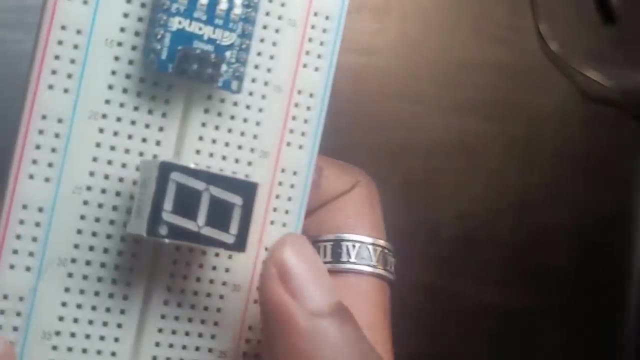 At the very, very left. Let me just again unplug my Arduino so I can get it closer And all I need to do is what? Connect the G right here. Let me just go over right here so you can see it: I'm going to connect the G. 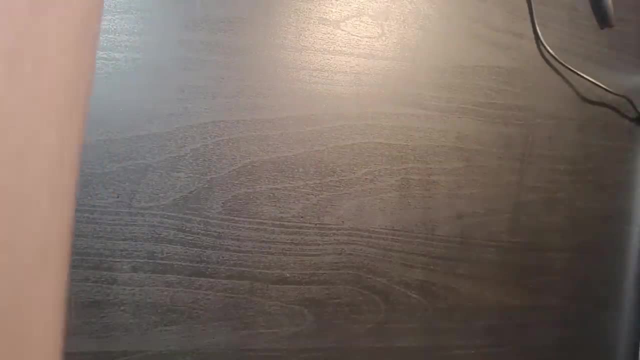 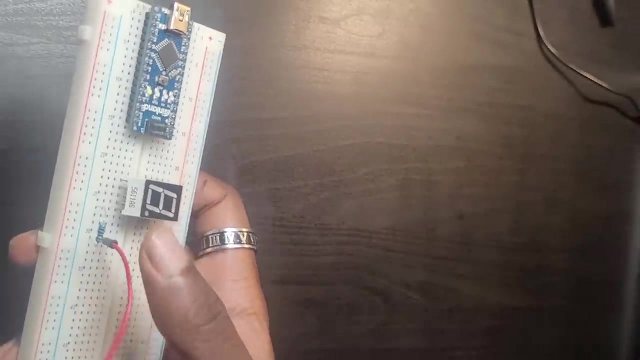 And then I have a wire. Let me just get a wire right here. Okay, I have a wire right here, Okay, But first let me connect the common one. What do I have I'm using? what A common cathode. 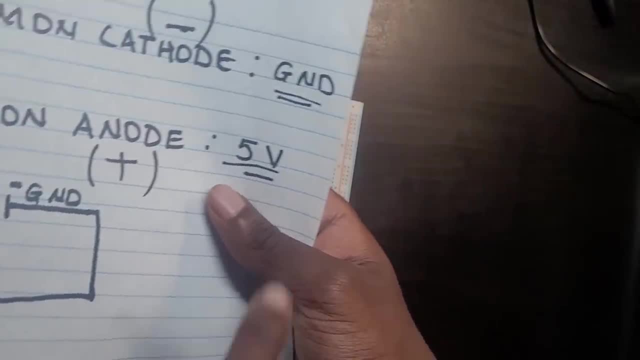 So it's going to have what. When I'm using a common cathode, it has what It has: a common GND. Let me just connect that The GND is found in the third leg, So let me just do that. 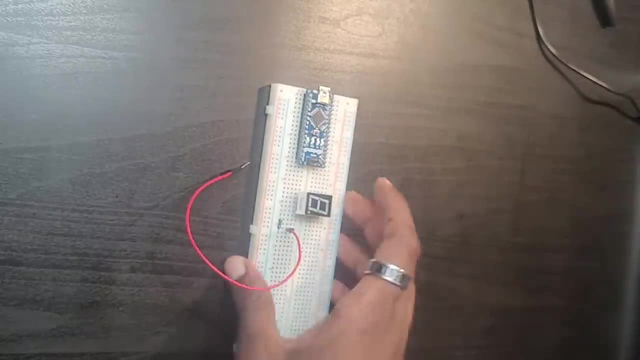 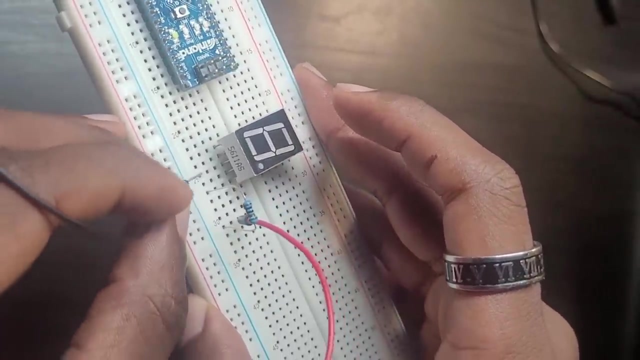 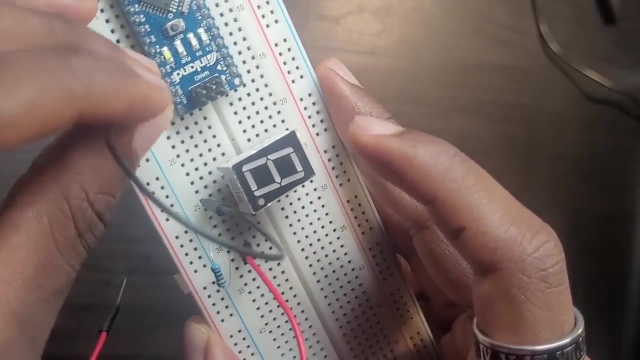 So let me bring a black pin for the GND. Let me bring a black pin right here, Count one, two, three, And here we go, There we go, Connect this to the GND. Let me just do that, And what I'm going to connect it to is a what. 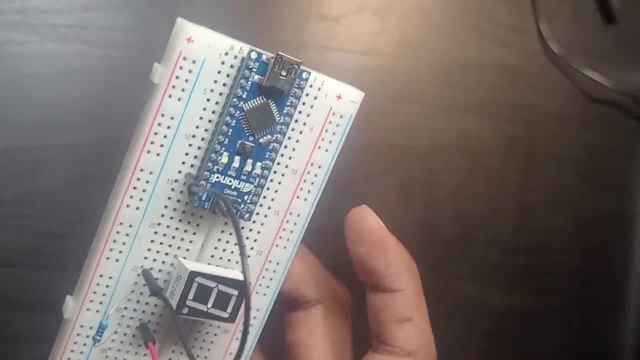 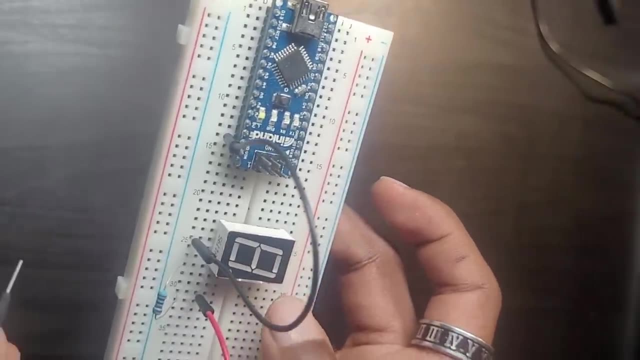 I'm going to be connecting it to a pin right here. Let me just connect it to Five volt for now, just to show you how it works. But I'm going to be connecting it to a pin when we're working with a project. 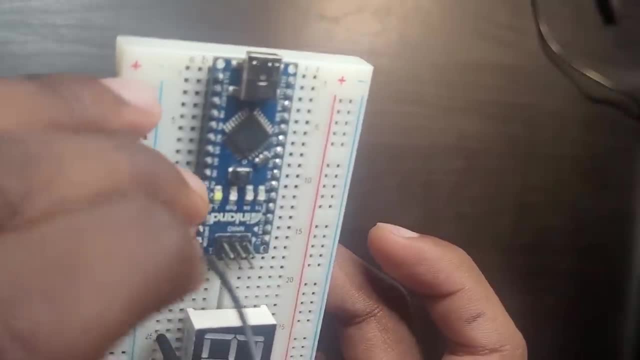 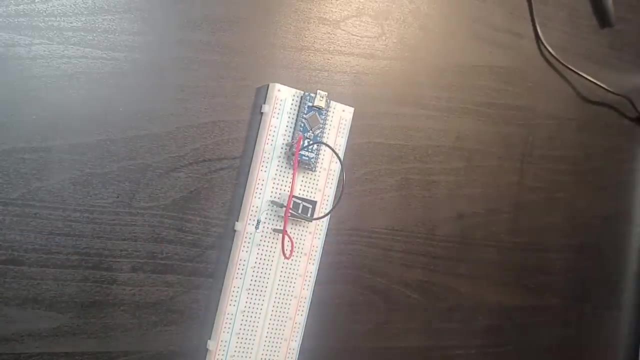 So, just to show you how it works, let me just connect it to a five volt. There we go, Connect it to a five volt. And now what do I expect? The G, the G to what? To light up, The G is found in the middle. 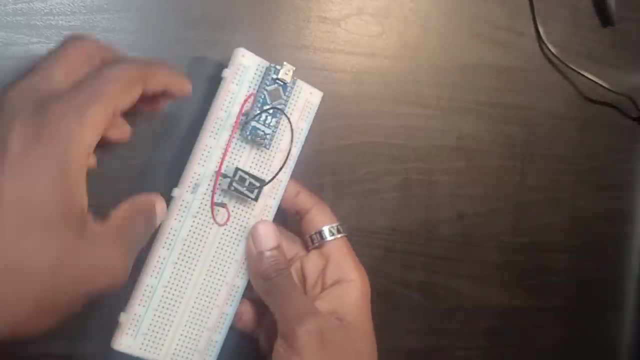 It's the middle segment. It's the middle segment, So I expect this to light up. Okay, The resistor should be intact. I'm using a 1000 ohm resistor. You guys can use anything between 500 and 1000 ohm. 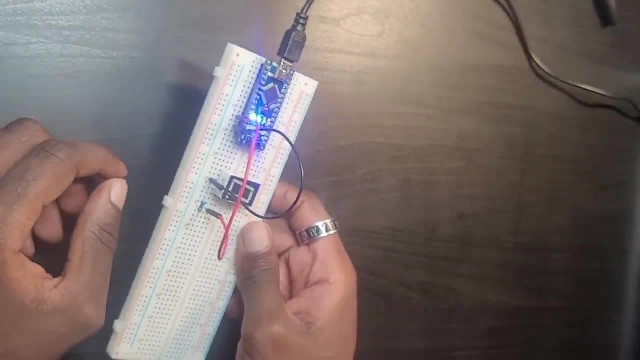 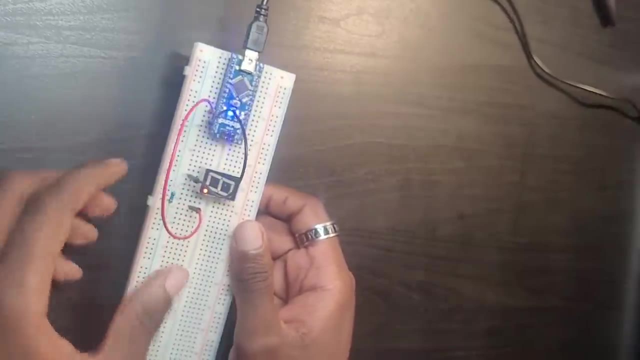 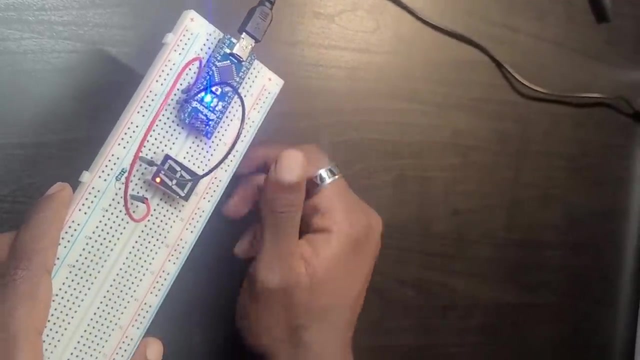 And this should be working, hopefully. Okay, Can you see that? Can you see that? What's happened? The common, the common, uh sorry, The common, capode is right, but what happened was: what did I do wrong? 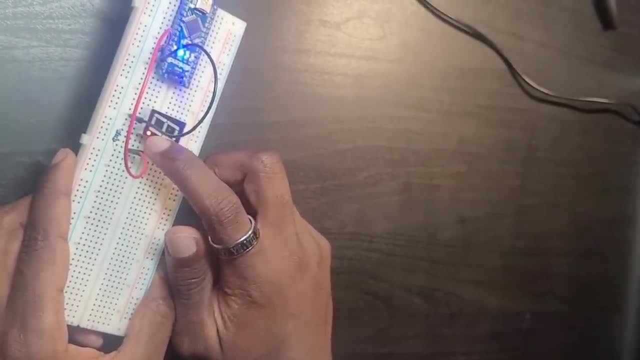 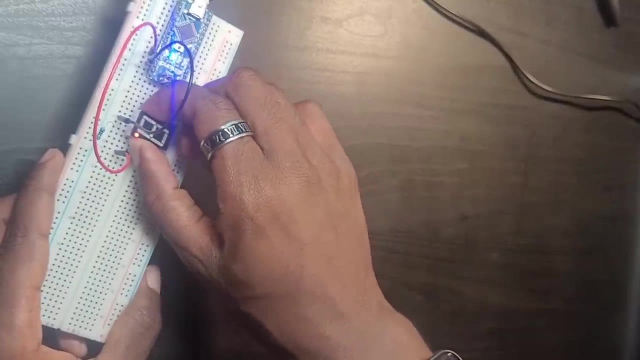 I got the decimal point light up. instead of what, Instead of the, the G. what did I do wrong? What did I did was I flipped it. Okay, What I did was what: I flipped it. I was supposed to put it like this, supposed to flip this like this. 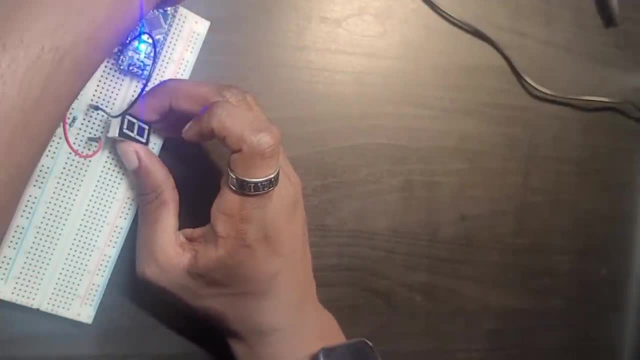 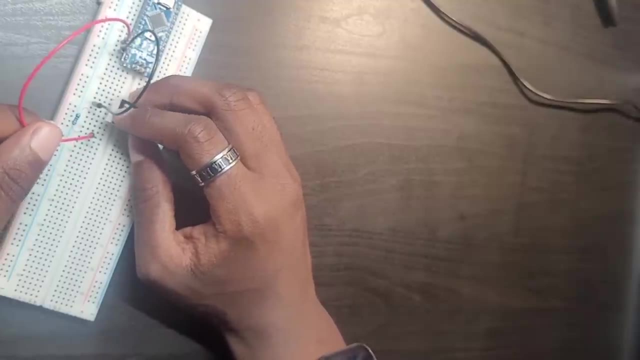 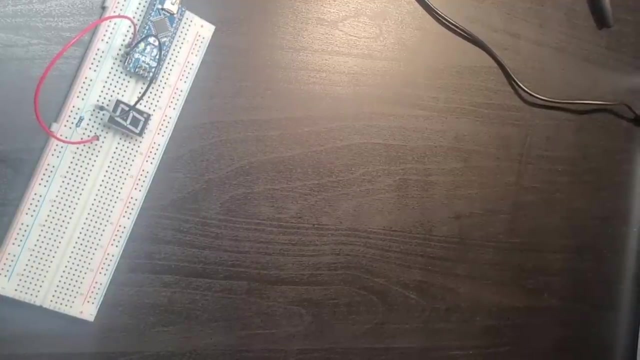 The decimal should be here and then put it down like this: first Let me unplug my Arduino, because again I don't want to get the pencil wrong. right, I think there we go. That should be it. Excuse me, All right. 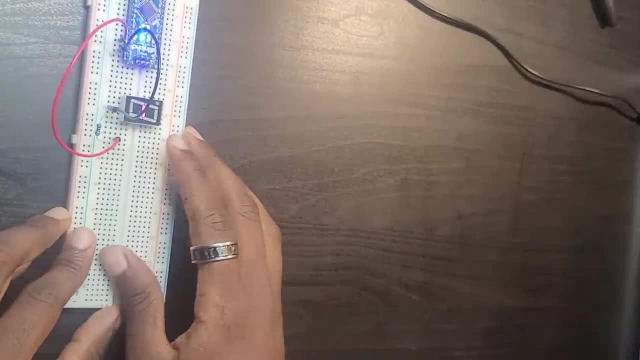 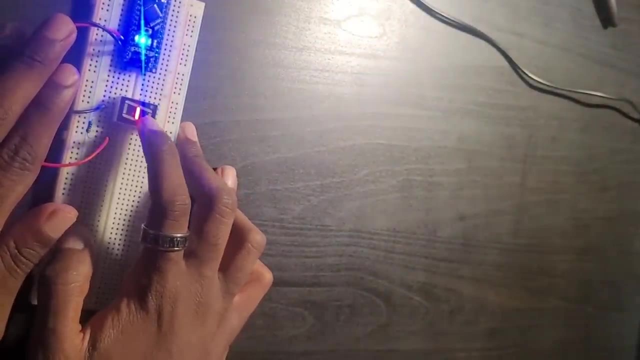 So now let me just plug back the Arduino. There we go. Now it's working. Let me just turn off the light so you can see it better. There we go. The middle, what the middle segment is lighting up, Nice. So now let's just go to the ones who have common anode. 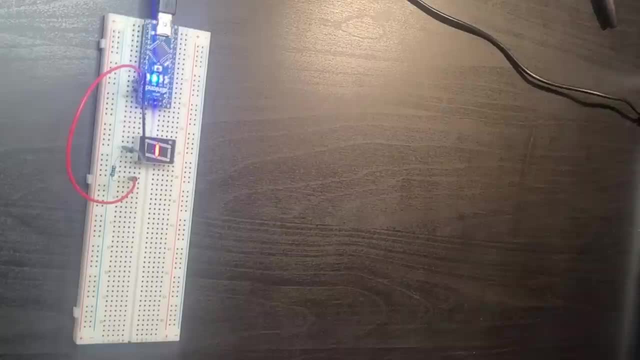 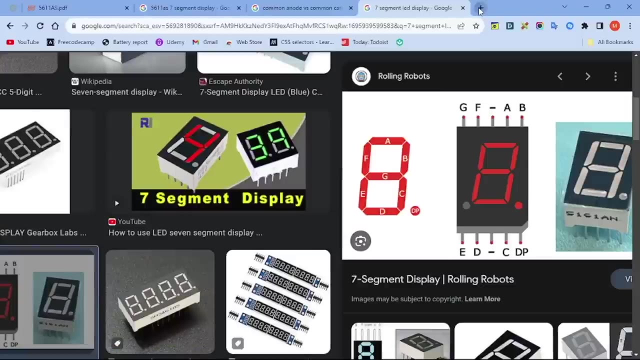 Let's see how you guys can actually do it. Let me just check that. And in the next section we're actually going to build the project with it. So let me just go over to my screen again, because I don't have specifically. I don't have, uh, my own, I don't have uh. 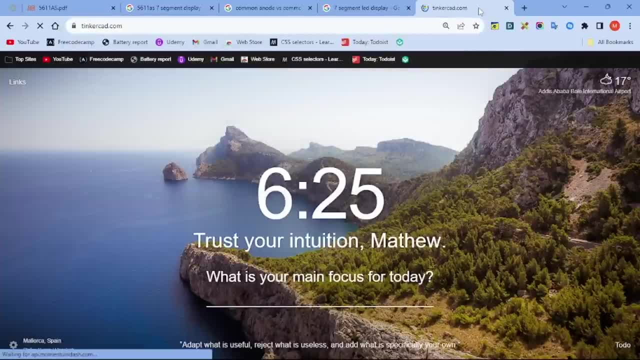 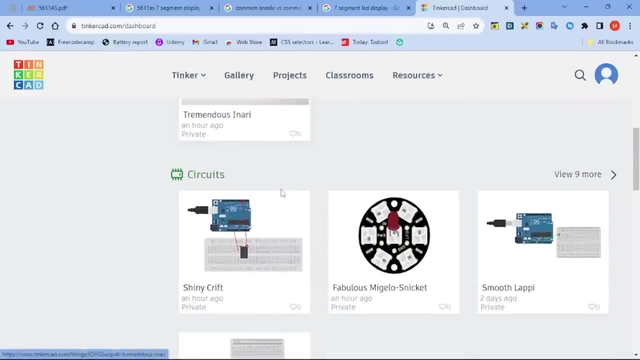 let's go to my Tinkercad right here. I don't have a- uh specifically, I don't have a. I don't have an adult, a common adult seven segment LE display, So I'm going to have to use a digital Arduino. 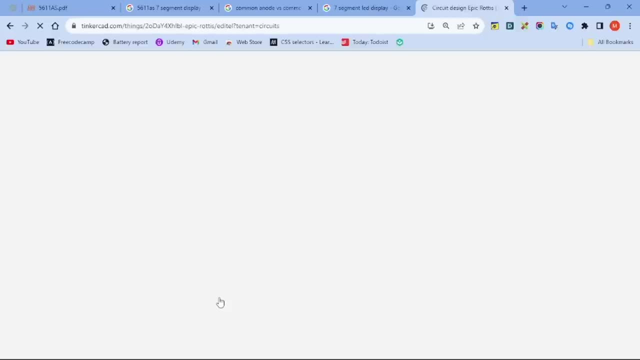 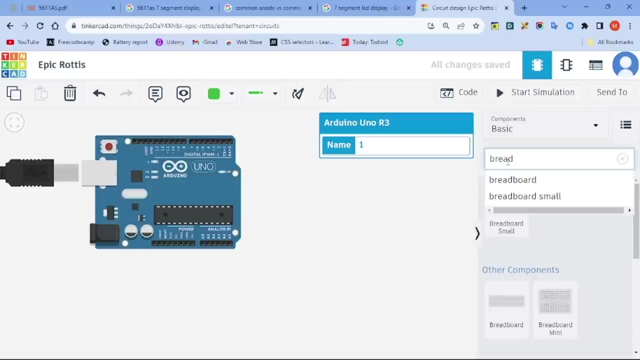 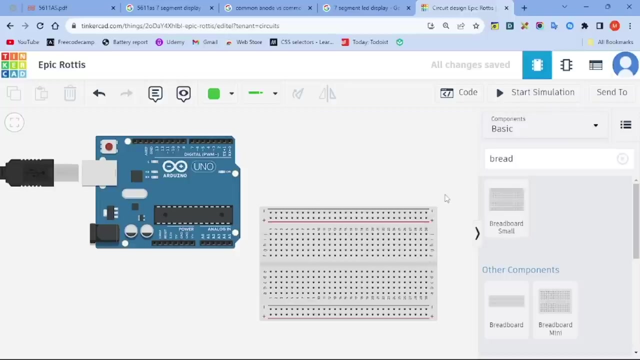 You just create that. It's going good. Now what I'm going to need is an Arduino. Get an Arduino. There we go. What else do I need? A breadboard- Right, I can get a small one for now. I'm just trying to light up what a single display that we're going to go to our project. 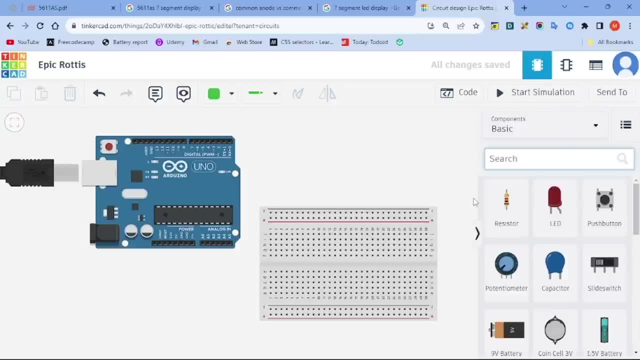 Okay, Now what do I need? I need a seven segment. Let me just write it down: Seven segment, seven seconds. I'm not getting anything, just seven segment. There we go. Seven segment display. Okay, So I'm going to set it to. what a common anode right here. 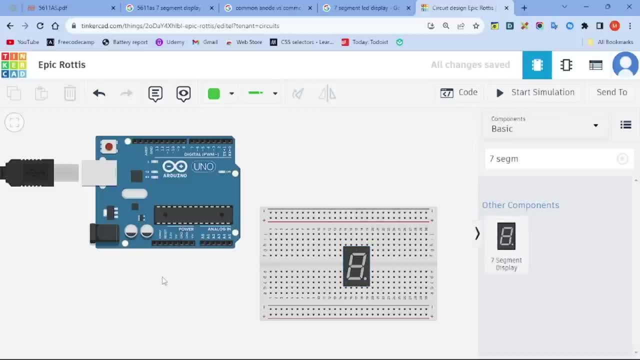 So you guys can Actually see how it's done. So they said again: a common anode. What do we have? Let me just bring back the paper. I'm not going to need this anymore. Let me just bring back the paper: common anode. 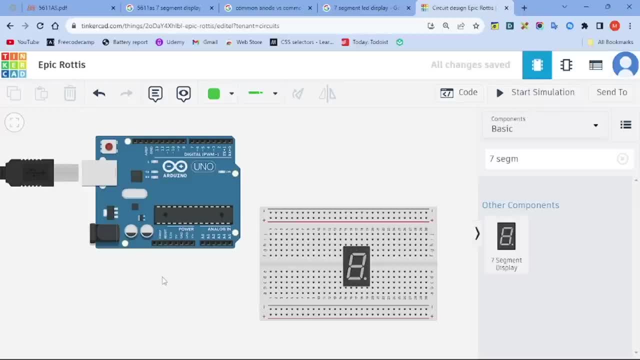 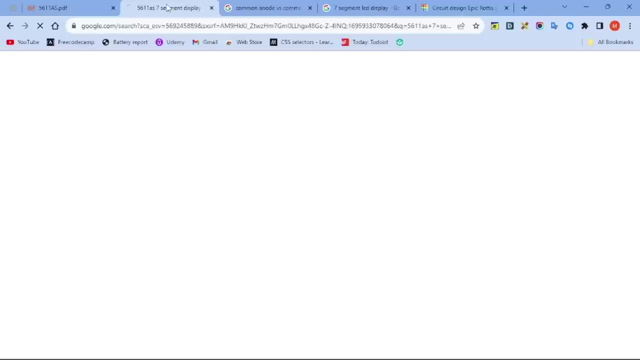 We can have a common five volt pin. Okay, So let me just connect the common one right here. So I said again, we have one thing to always keep in mind. by the way, we just go to the image. Do we have the image? 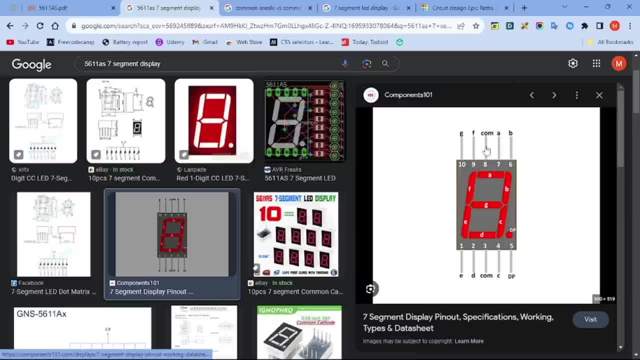 Okay, There we go. What we have to do is connect to one of these again. Okay, One of these. we don't have to connect both of them. Okay, We don't have to connect one five volt and another five volts. 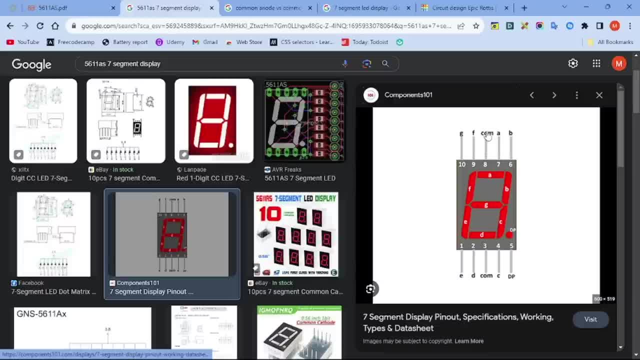 All we have to do is connect one of them. Okay, All you need to do is what connect? one five volt, or one five volt that comes to a common anode. when it comes to a common cathode, What do you need to do is what connect to what? um one common, what GND, not like two GNDs. 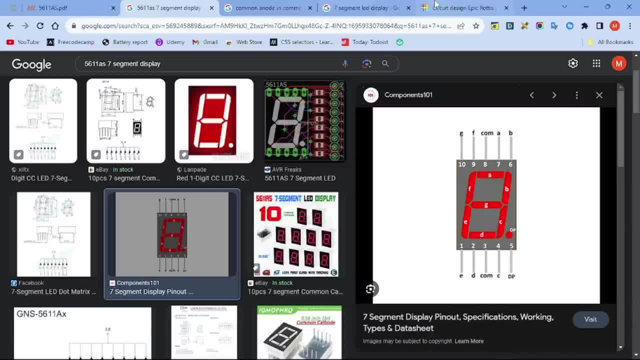 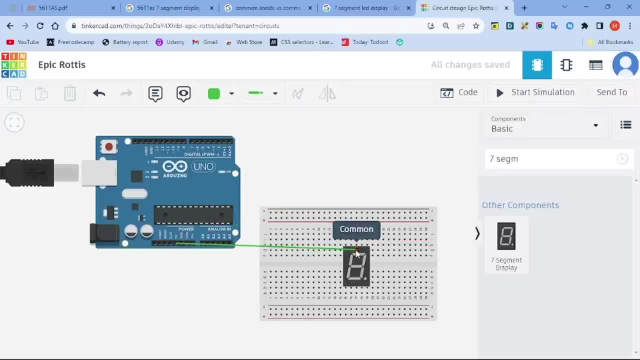 All right, So you can choose either one and just connect it. Okay, All right. So with that in mind, all you need to do is I'm going to connect the five volt right here. So the third leg, the third one, is here: the common. there we go. 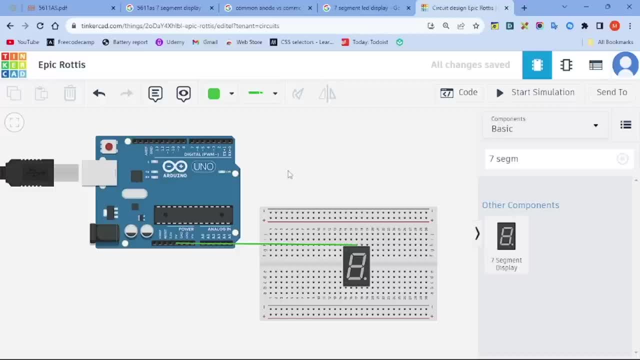 Once I'm done doing that, I'm going to use a resistance on the GND. Let me just get a resistance. Let me just get a resistor resistor. There we go. Got a resistor. What value? one kilo ohm, basically meaning 1000 ohm. 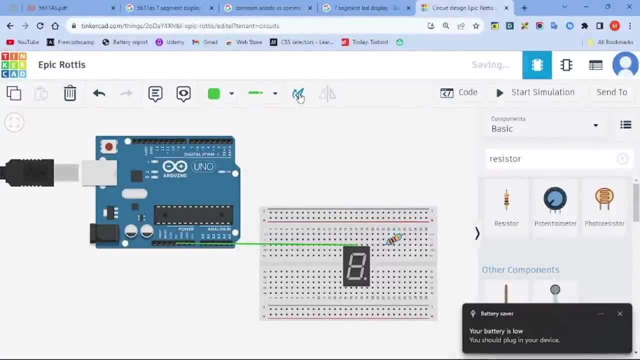 Let me just rotate it. Let me just rotate it so that it fits me. Let me try it. I'm going to light up a different segment here. Let me just try to light up this one. I don't know what, what this one is. 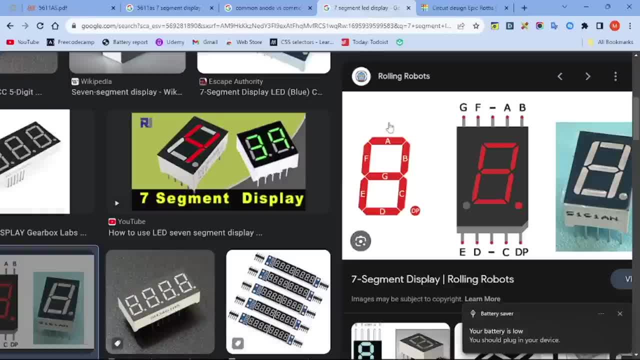 It's B. Which one is B? Let me just see which one is B. Okay, So I'm going to be lighting up this part. I'm going to be lighting what? what? the right one, the right, the right upper one, the right upper one. 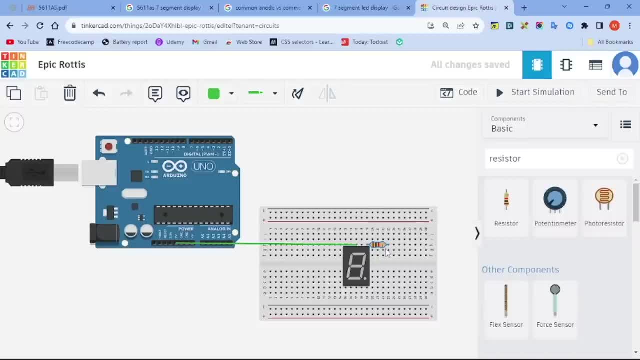 Okay. So let me just go here and I'm going to need my. I'm going to be using what. I'm not going to be using: GND, Don't get that wrong. Okay, I'm not going to be using GND. 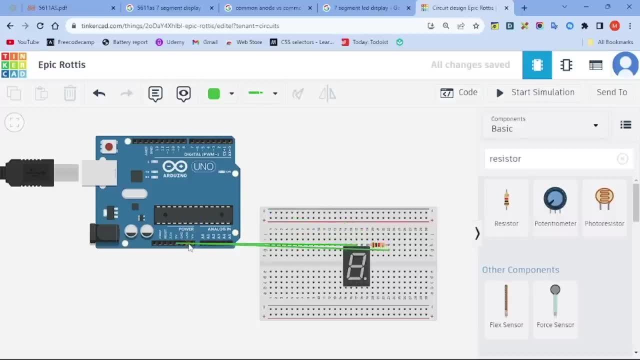 I'm going to be using digital paints. Yes, I can use a GND- GND for now. Let me just try to use a GND for now. Let's see what happens. I've never used the GND with that. 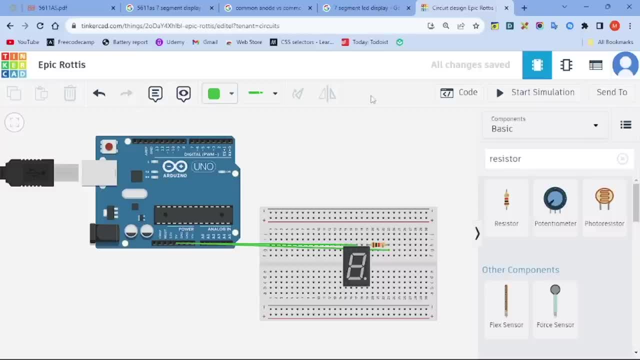 Yeah, Let me just just land it on GND, Let's see what happens. actually, I think it should light up There. we go, It lights up. As you can see it, it lights up. So we're going to do again. 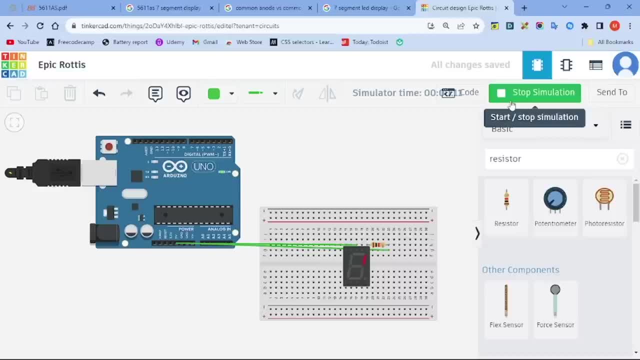 So right now, what we did is light up a common anode and a common cathode. So for those of you again, we're going to follow along with a common anode. I'm also going to again provide you with the course right here. 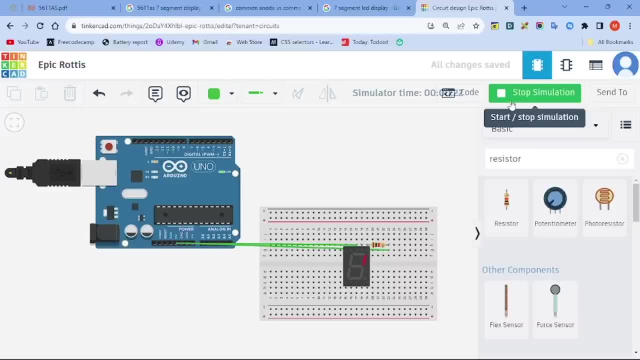 So you guys do not need to again go to another YouTube video or another documentation to understand, because I'm going to be covering both common anode and common cathode. Okay, So in the next section we're actually going to build a project. 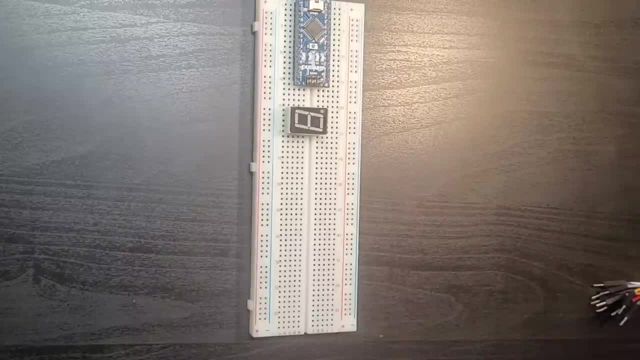 So see you then, Okay. So what do I want to do for this project? What I want to do for this project is build Somewhat of a simple timer, So I want it to count from nine all the way up to zero. 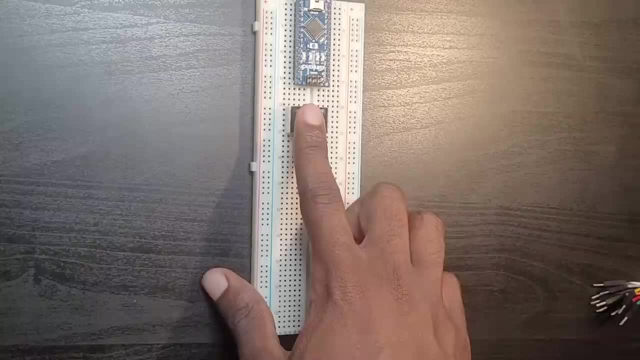 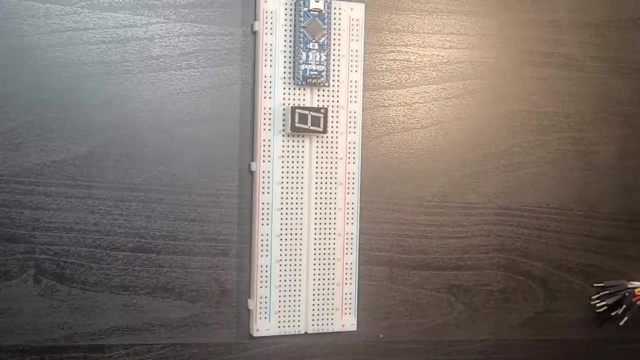 So I want it to go nine, eight, seven, six, five, four, three, two, one and end it at zero. Okay, So we just want to build somewhat of a what personal timer, Okay. So first, how do we do that? 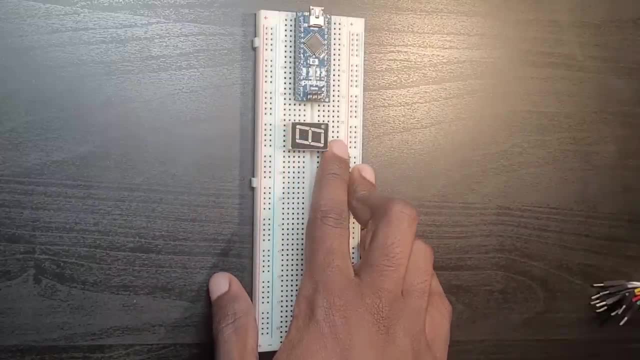 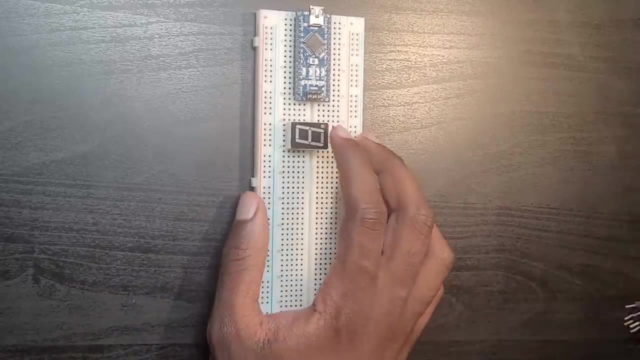 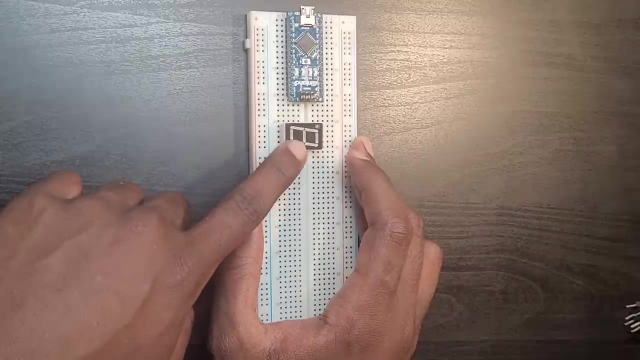 So first, what do we need to do? We need to plug all the components here. Well, obviously we did not plug any components and then we're going to go over to code, So let's first plug All components, Okay, So again, they said the third one. the third one is what? the third one is the common ground here? for me it's a common cathode. 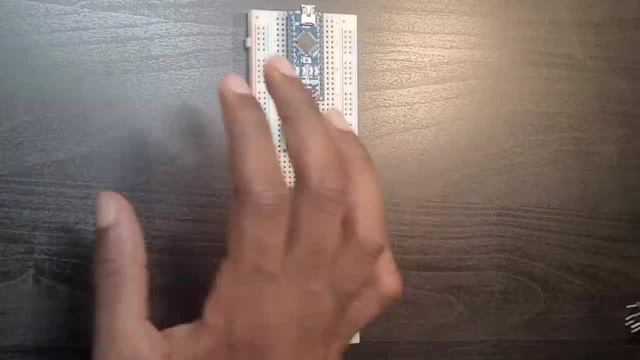 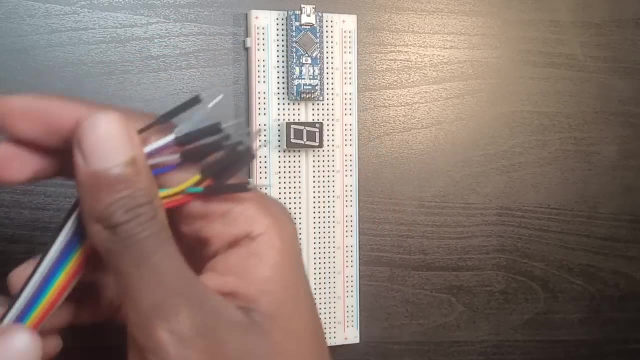 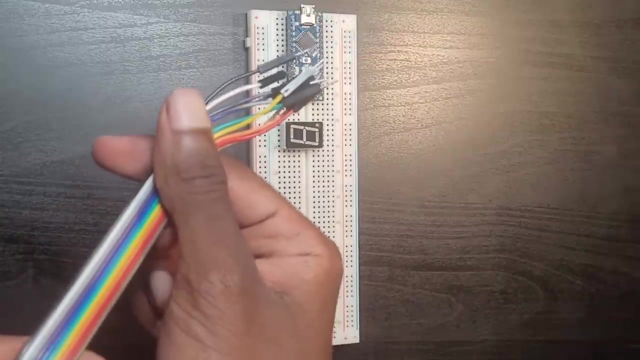 So I'm going to be what using? what a common, what a common GND. Okay, That's all we said. All right, So let me just get this over with and just bring this. There we go. So, instead of using normal wires, what I'm going to be using is strapped on wires, wires that extract each other. 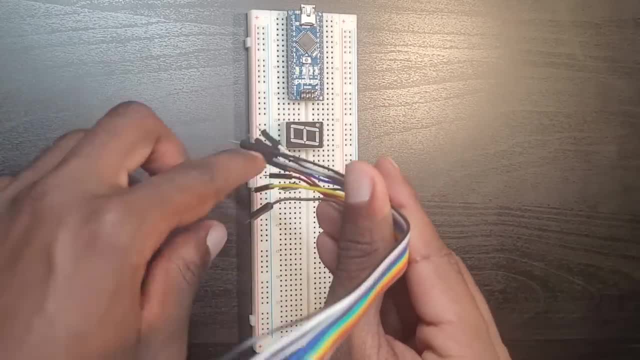 So when you look at them, they're strapped to each other. It makes things way easier for me, as all I need to do is connect. connect to continuously, and then what? and then all I have to do is connect to continuously. here too, 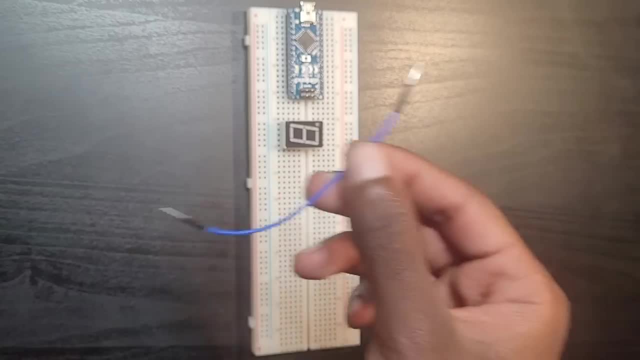 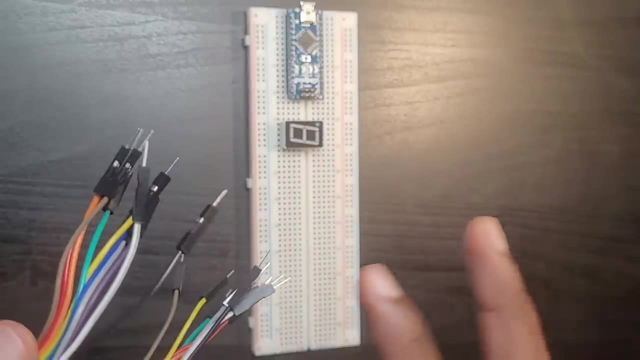 So it's going to be way easier than using again normal wires- Okay, Than using normal wires. But if you don't have any of these strapped, these strapped type of wires, the normal wires are perfectly fine. They don't make any difference in terms of conductivity or anything. 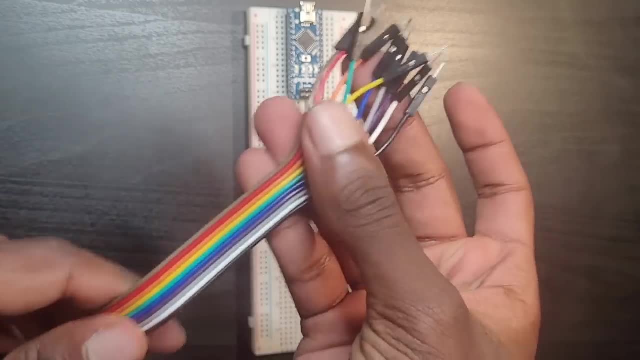 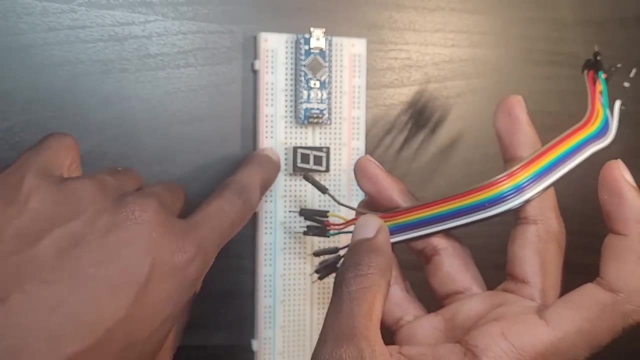 Only. the only reason I'm using them is I want to introduce new components to only that too. but it makes it way easier, Because once I put them right here, let's say I set up the five pins that I'm supposed to be connecting here. 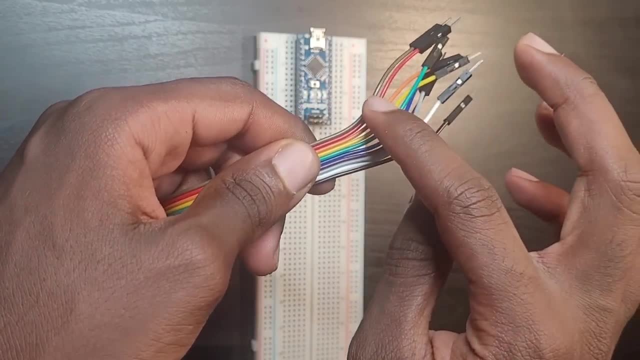 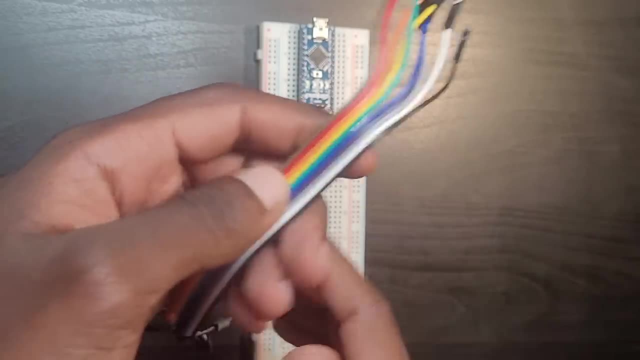 Once I set up the five pins right here, all I need to do is what? See it relatively from here. So I go- brown is first, Okay, Brown is here, and you know- and go right here- Brown is here And then relatively tell what the distance from here. 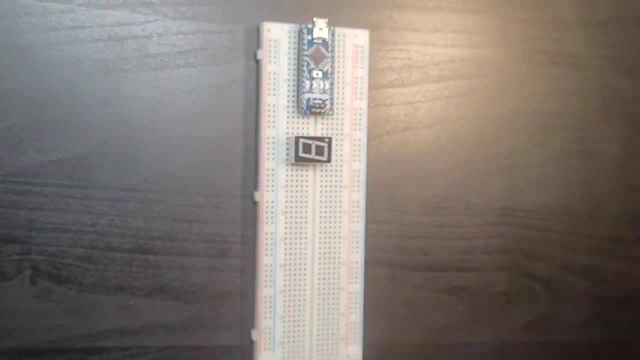 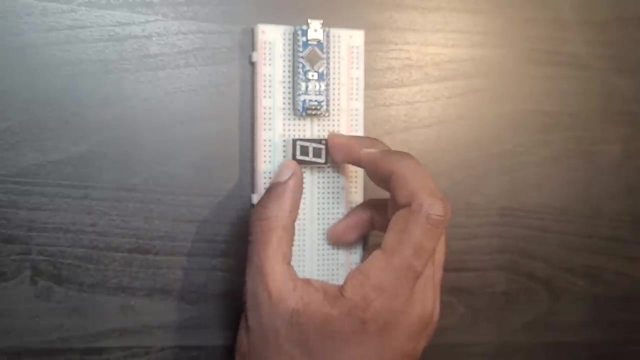 I don't have to go the whole way back here just to tell which pin is connected to which pin. So it makes it way easier, especially when connecting what? when, when connecting wires that are closely to each other, right, You have five pins to connect to. 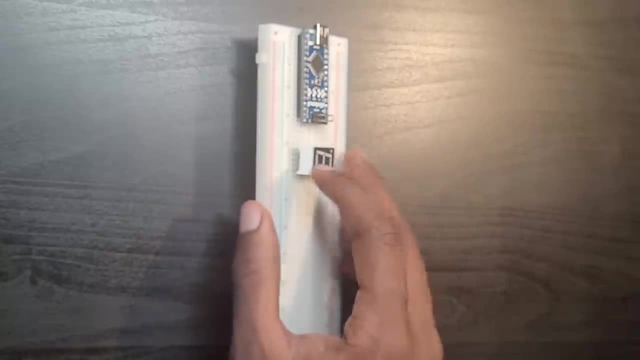 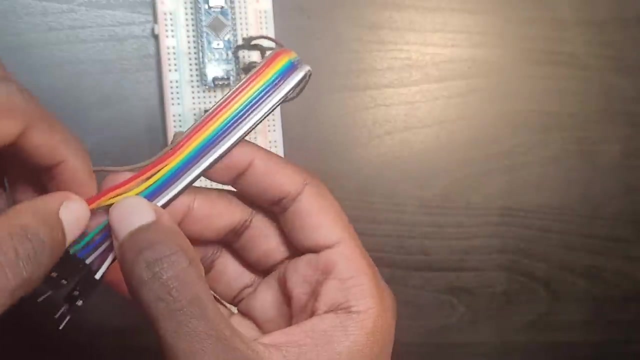 Let me just check it right here. Five pins, right, I've got five pins to connect to right here and five pins from here too. Okay, So let me just get started. So let me just arrange this so that it matches the color. 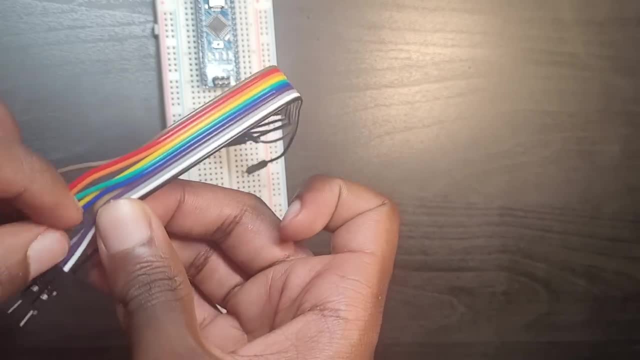 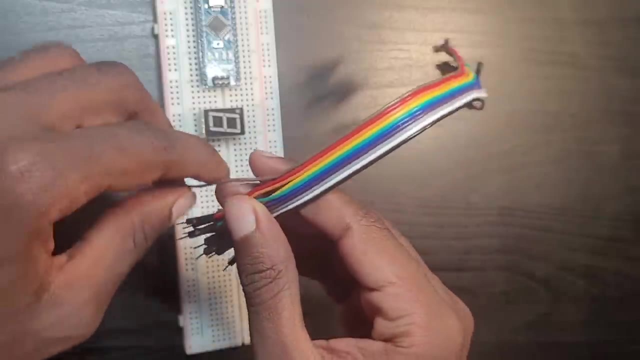 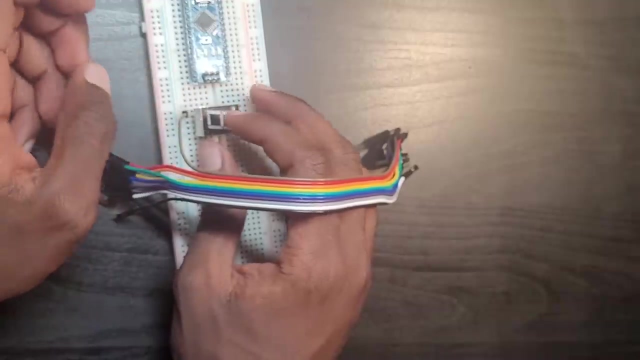 There we go. Right, Seems to get purple. needs to be in the middle right here. All right, there we go. Simple arrangement: Now you can get started. So let me just start with brown right here. All right, what did I do wrong right here? 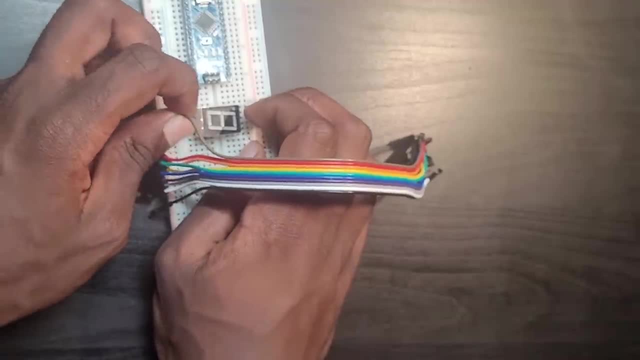 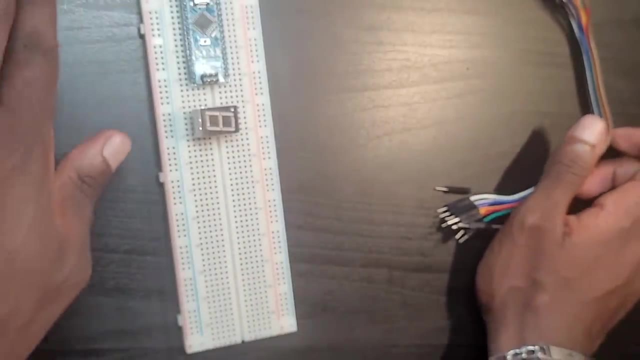 I forgot to put my resistors first. resistors do what they come first. Okay, So obviously I have to connect my resistors first, and then I'm going to be connecting my wires, So let me bring my resistors right here again, I'm using 1000 on resistors. 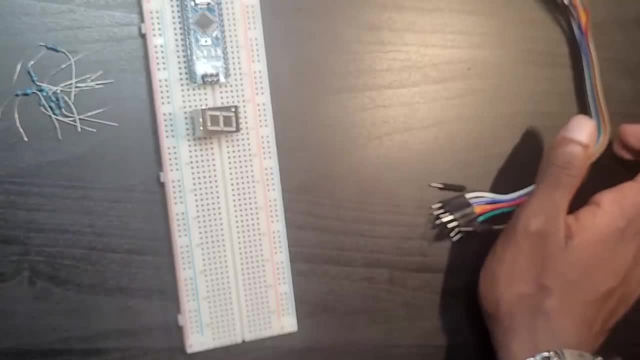 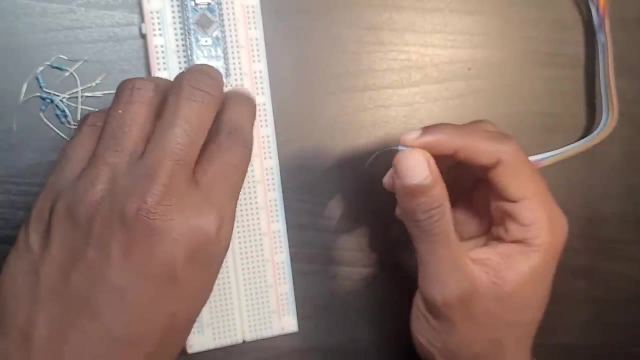 Okay, I have a collection of them, 1000 on resistors. But again, you can, you guys can obviously use anything between 500 to 1000. Okay, So it doesn't directly have to be 1000. Okay. 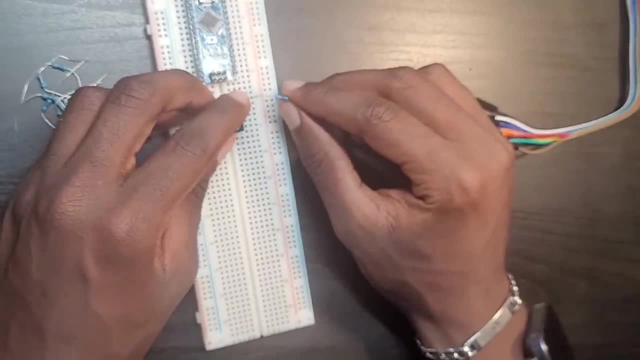 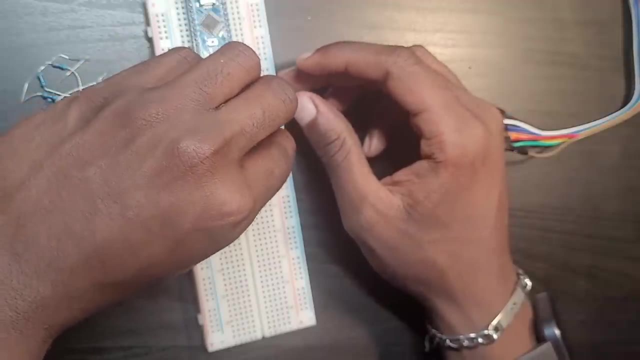 Okay, So let me just put this here. What I'm going to do is I'm going to move the resistors across. Okay, that's what I'm going to try to do right here. There we go, Try to move it across. 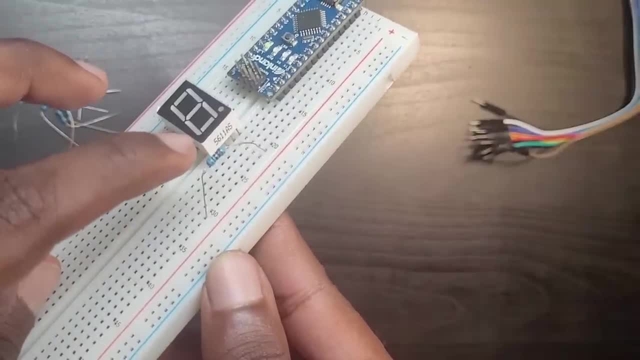 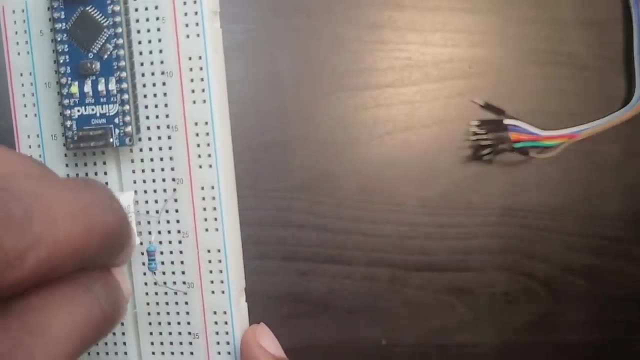 Let's connect the first one right here. Focus here. There we go, It's connected. Now I keep on bringing resistors. first Let me connect all the resistors, and then I'm going to continue and connect it to the wires. Let me just do that. 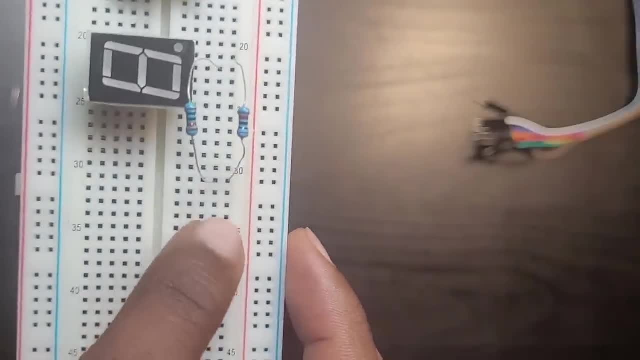 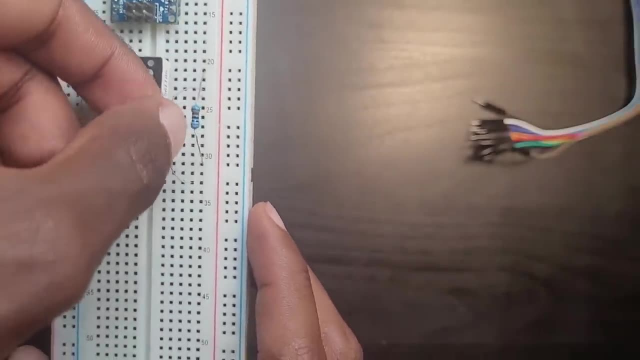 Okay, You see what I did right here. I connected a different, the second pin, but obviously they ended up in the same row, So all I need to do is again widen it a bit, and there we go. Aim for it, Okay. 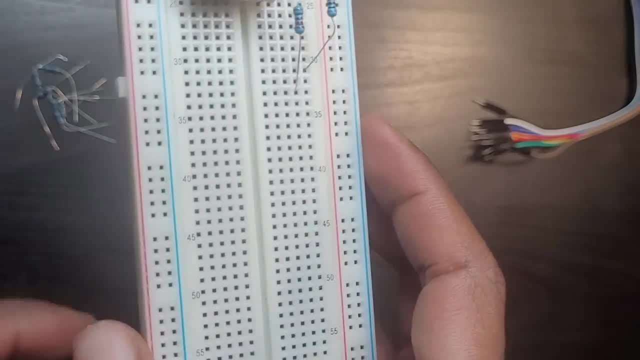 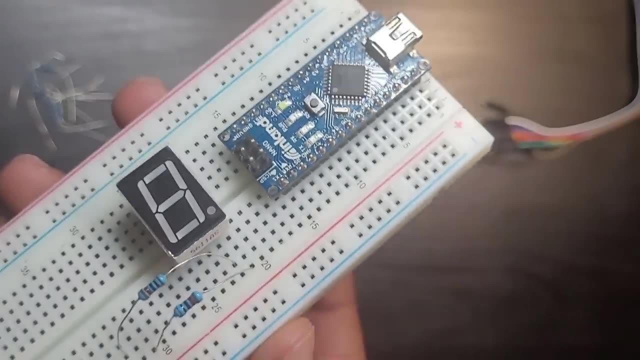 I pushed it a bit. There we go. Come on, It's a bit of a hustle to actually connect them when you have a little amount of space. Okay, So it did connect. Yep, It did connect right here, All right. 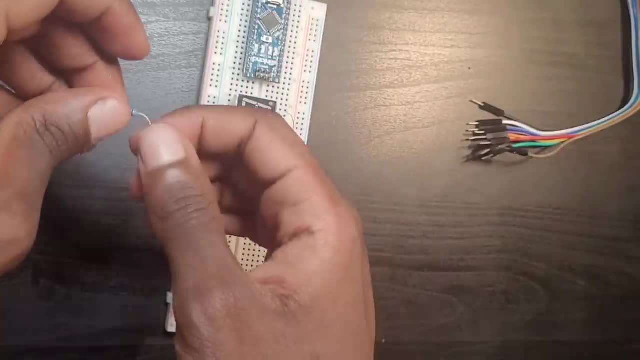 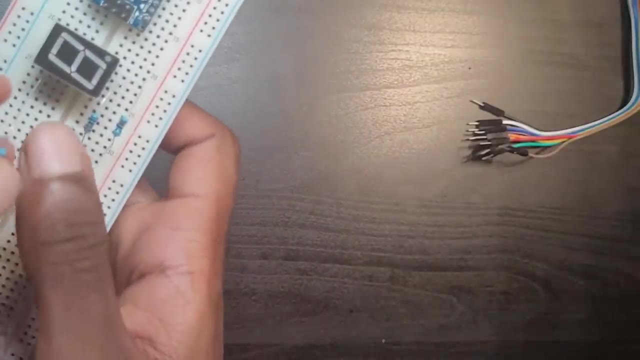 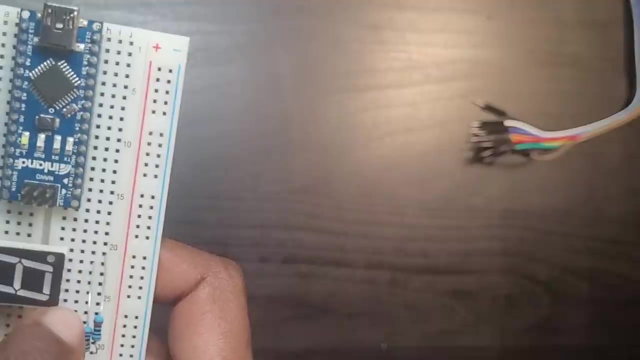 Nice, I'm going to bring another resistor. Let me try to find the one that is wider. Let me just widen it up myself. All right, Now the third one. what am I going to do to the third pin? As we said again, when you look at the diagram, we have two common pins. 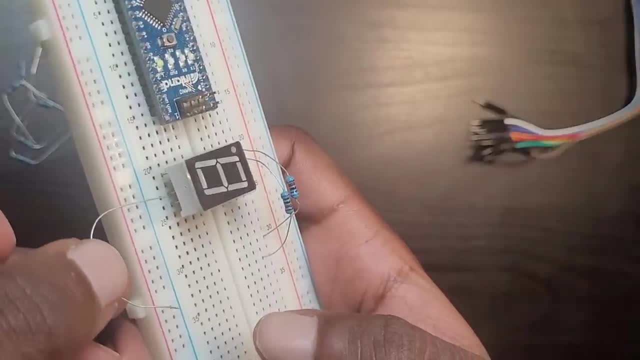 All right, We have two common pins. This is the third pin right here. It's going to be the common one. The third pin right here, just point it using my resistor. It's going to be what The common. The same goes here too. 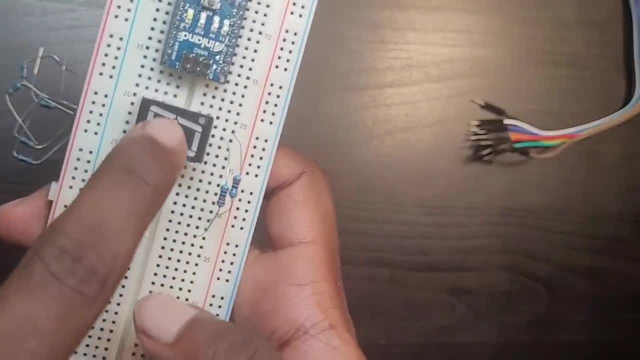 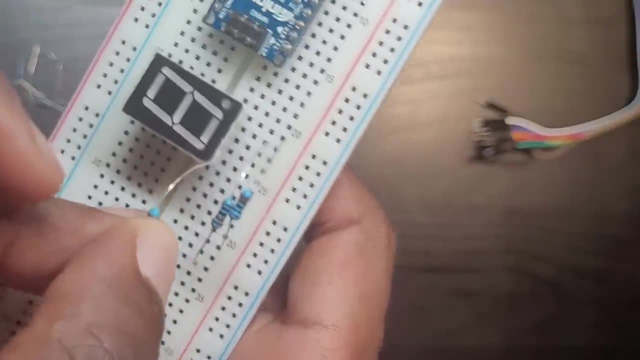 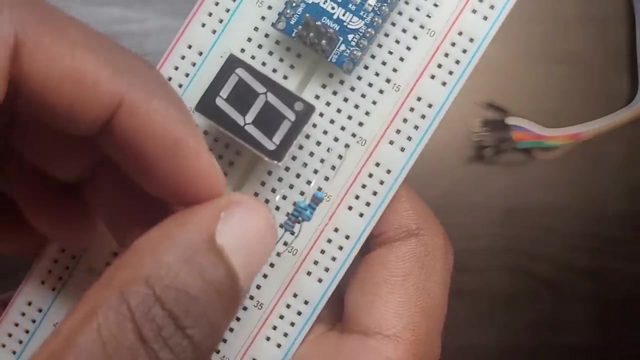 It's going to be the common. So, again, when it comes to the common, I'm not going to use any resistance. I'm going to be only using resistance. for what? For the separate segments here, all the segments. So let me skip the third one and go to the fourth one. 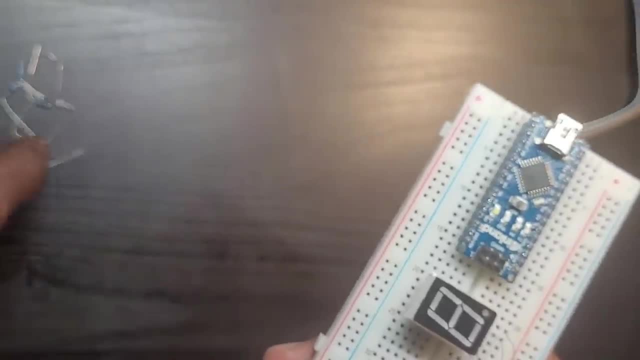 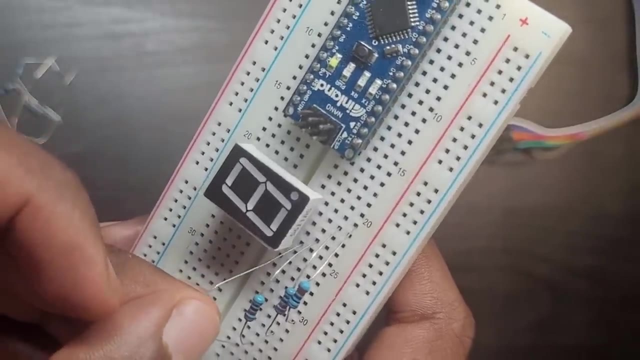 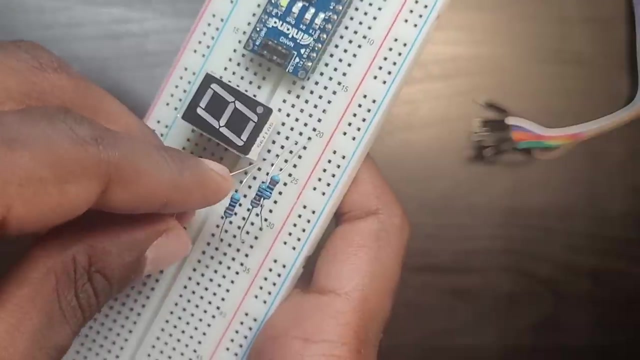 Okay, You need to be really careful not to connect the wrong pin, the wrong resistor to the wrong place. Everything can go wrong once you plug it, once you plug your Arduino, If you don't be careful. Okay, Wait Slowly. 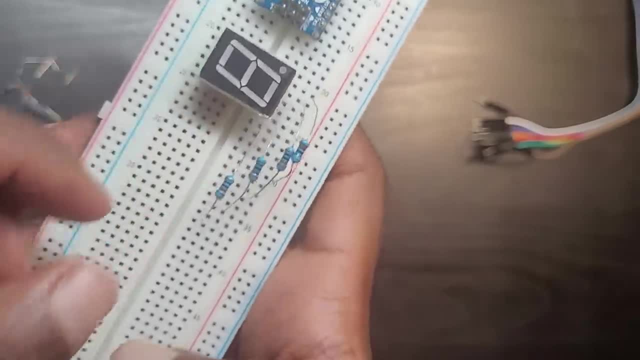 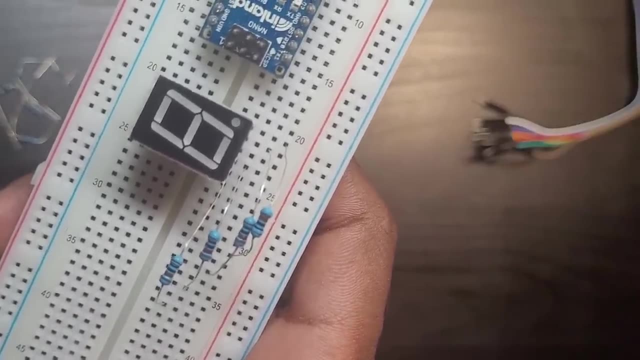 Let me let me wait in this a bit. All right, There we go Now. let me just check it. Okay, When you look at here, I connected one, two. I skipped the third. Now the fourth is connected and the fifth is connected. 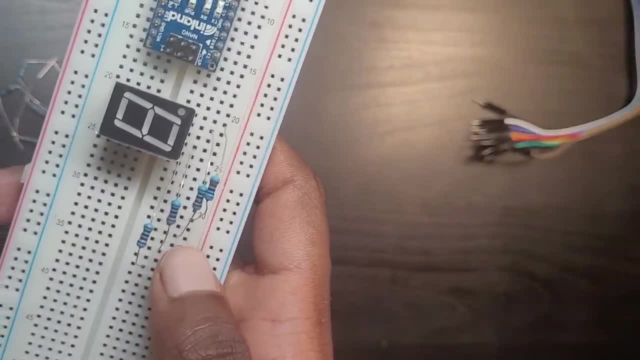 And all of them are not in the similar. they're not in the same row. I just want to keep that there. I don't want them to be in the same row. Okay, All right, They're not in the same row. 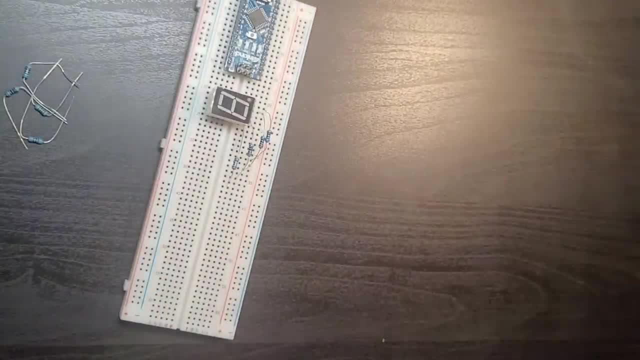 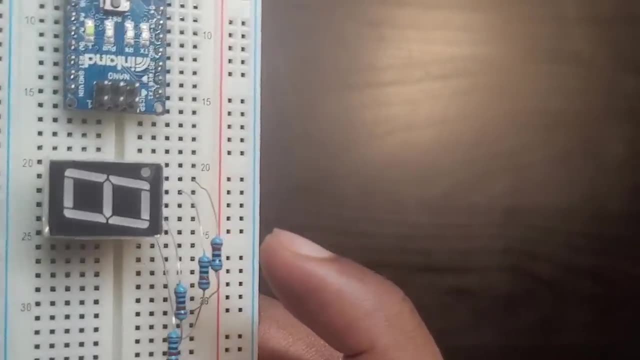 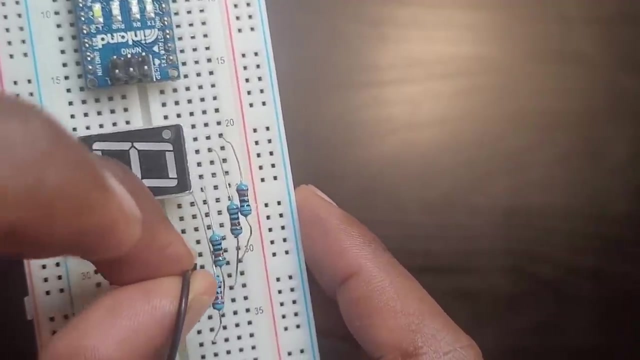 Now I can start using again these pins, So let me just do that. Just go here. It's a bit of a hard one when you're picking it, the breadboard up, It's really hard. All right, There we go. 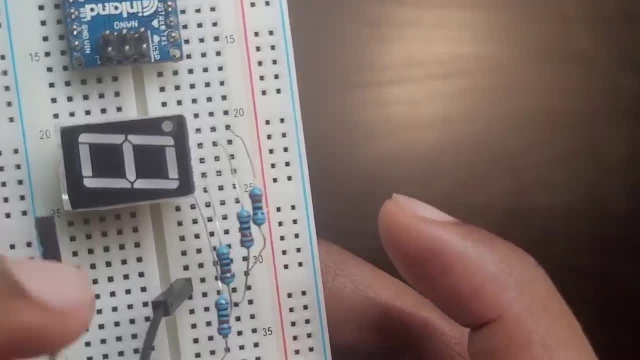 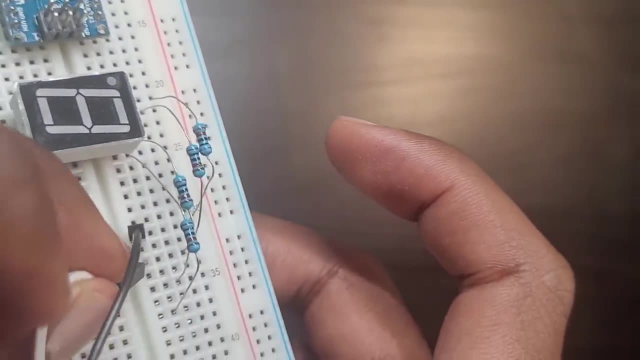 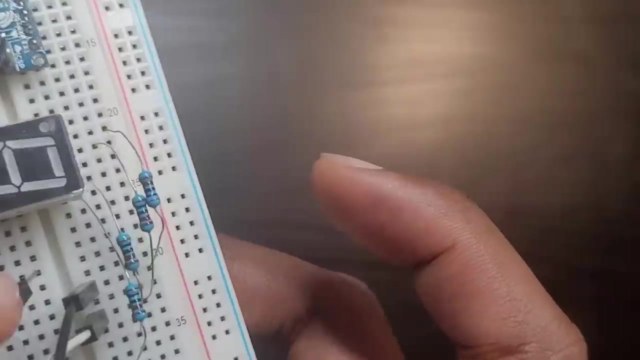 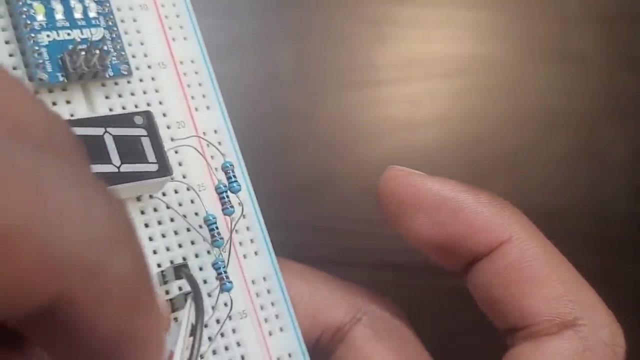 Connecting to the first resistor here. And then the next color is white. Let me go get white. Okay, I need to go here, All right. The third color is silver. Let me get silver. Okay, Let me just see that you guys can actually see it. 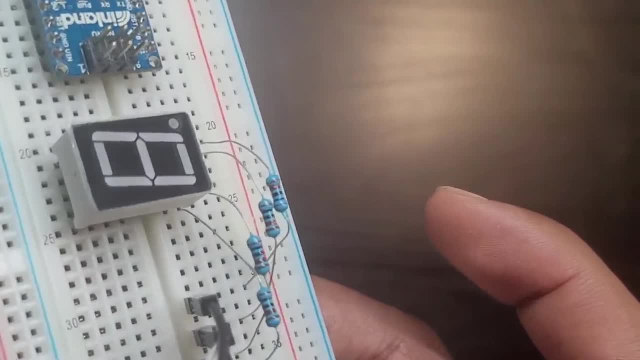 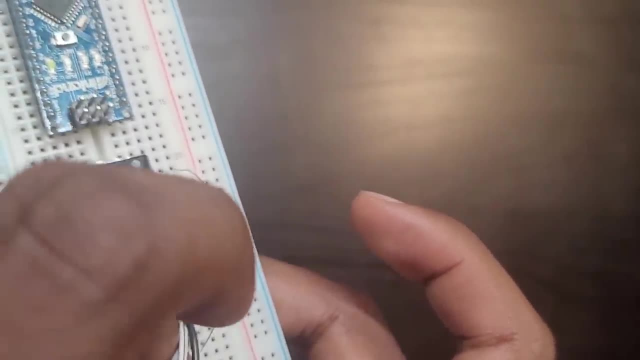 There we go. Can you guys see it? Yeah, We got connect the third one And the fourth resistor, The fourth and the final resistor from this side. All right, Let me connect this one. Obviously, what did I not do right now? 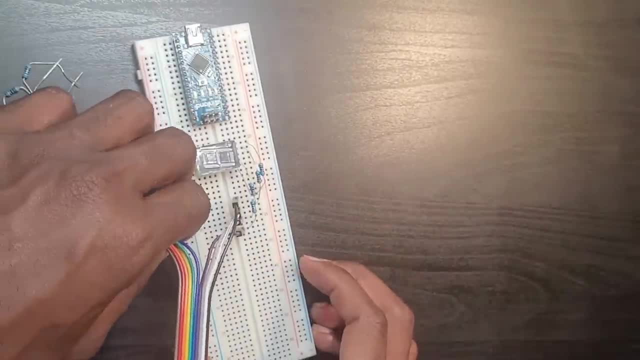 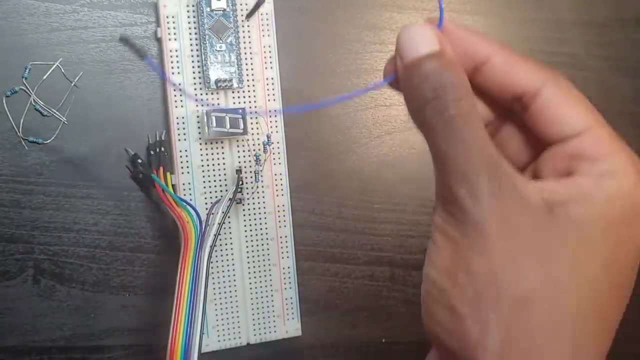 I did not connect my GND pins, So let me go over right here. Okay, Let me go over. Where's my GND pin? Let me just bring a separate wire for GND. Okay, I'm just going to bring a separate wire. 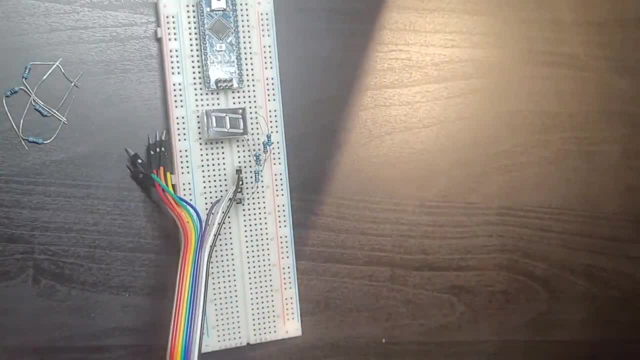 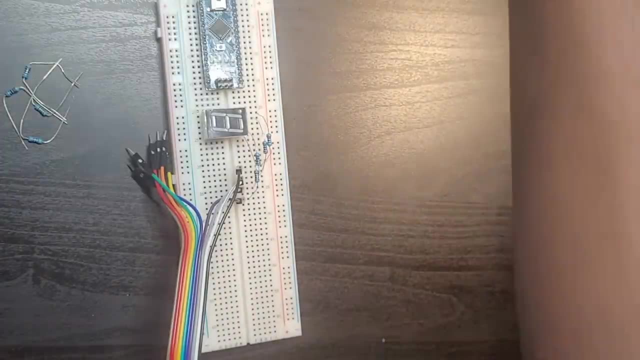 It would be preferred if I again bring the black one, because we use black wires to connect GND Just to maintain the code, if I can. if I have a long black wire Trying to look for one, Okay, There are no long black wires. 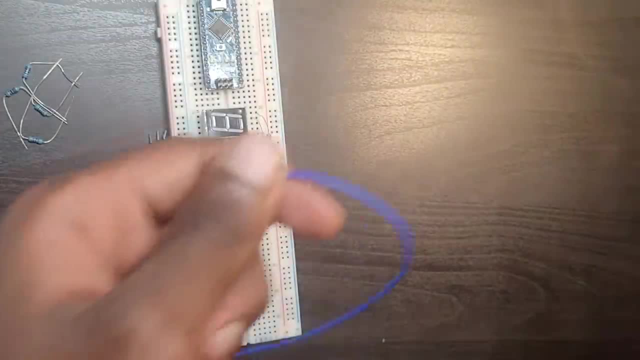 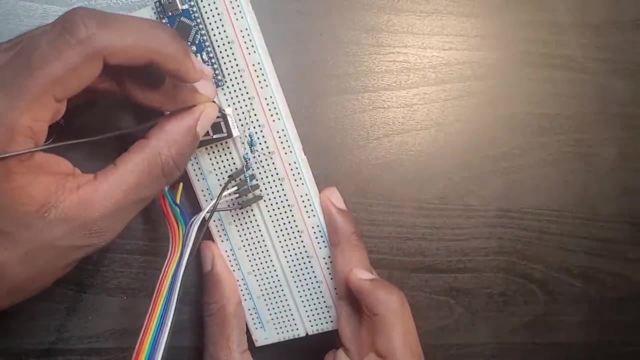 So I'm just going to use black. Okay, I'm going to connect the GND. I cannot find it, But I did. I think this one is long. Okay, There we go. Found a black long wire, So I'm going to connect the GND. 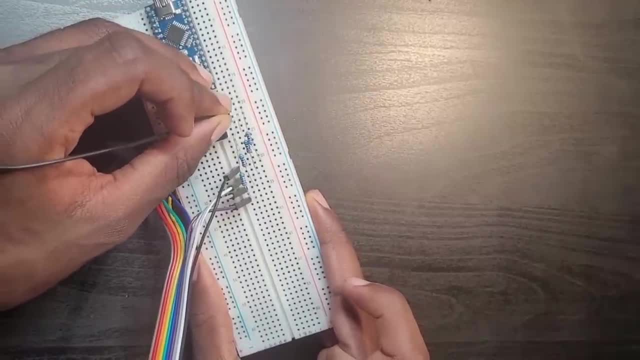 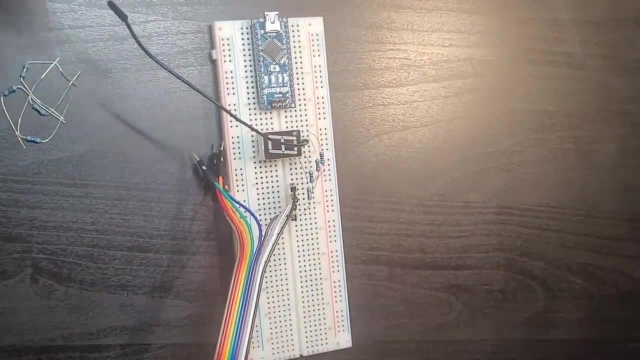 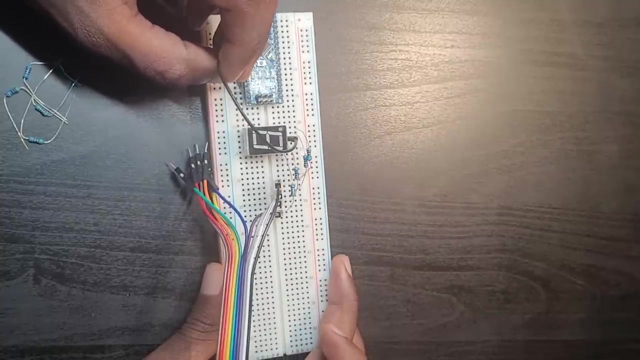 Let me just do that. It's supposed to be one. two: It's supposed to be right here. Okay, It's a bit of a hustle again. Let me connect this to the GND. We have a common ground pin. Just connect it to it. 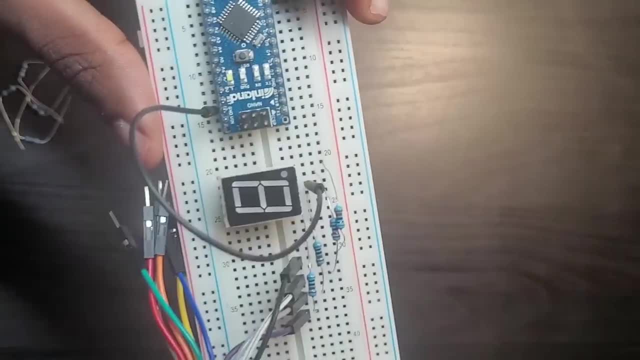 There we go, Connected it to GND. All right Now, obviously we have our wires from the other side. Now I don't have enough space here. As you can see, I only have one row of space right here. 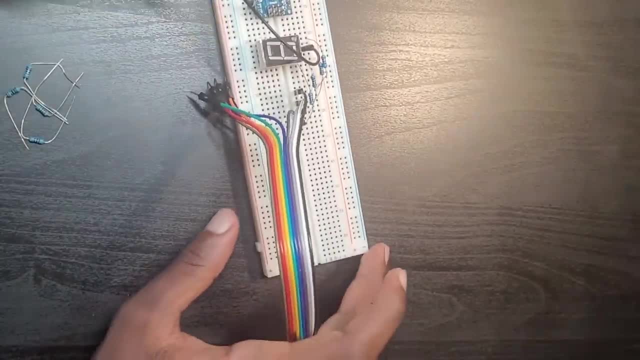 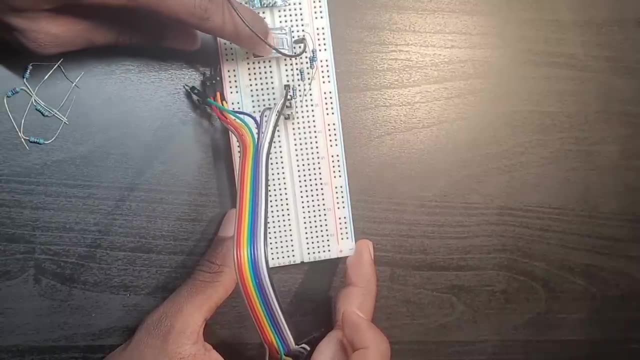 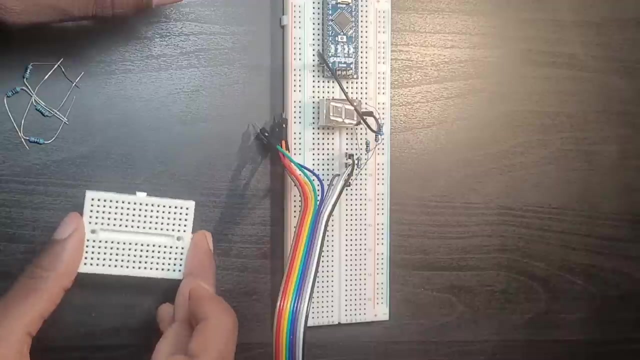 I have one column of space Because, as I said again, this LED is big. So what I'm going to be doing is, creatively- I think a creative idea is to use a smaller breadboard, So I'm going to be connecting it to what? 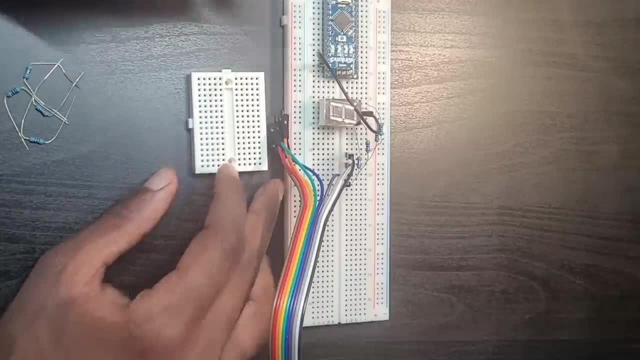 With the resistor across here, And then I'm going to be connecting it to the GND, And then I'm going to be using a smaller breadboard and connecting it here. It's better that way, So let me just do that. So let me forget about these wires right now. 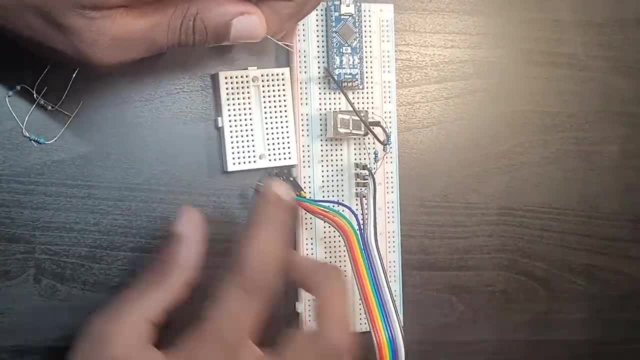 I'll just put them right here. Let me just make sure that I have the numbers intact. It has numbers on it, So I'm going to be referencing the numbers right here on the breadboard. Let me just bring it closer so you can see it. 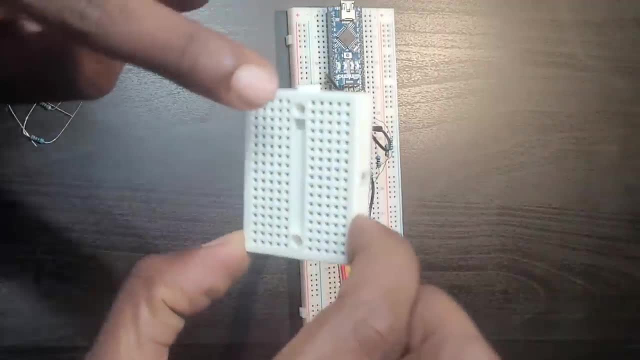 There you go. They have numbers One, two, three, And I want to again reference this one. Okay, So let me just do that. Just take off this one for a moment. It's a bit of a hard work. 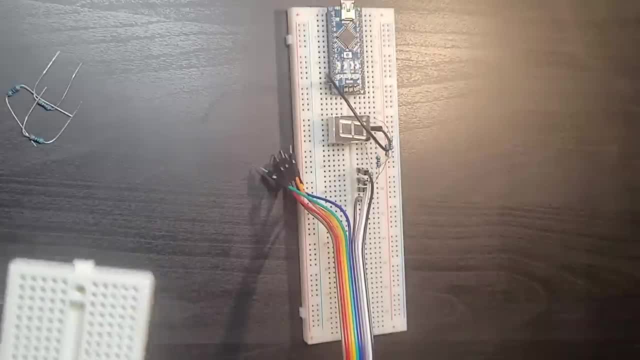 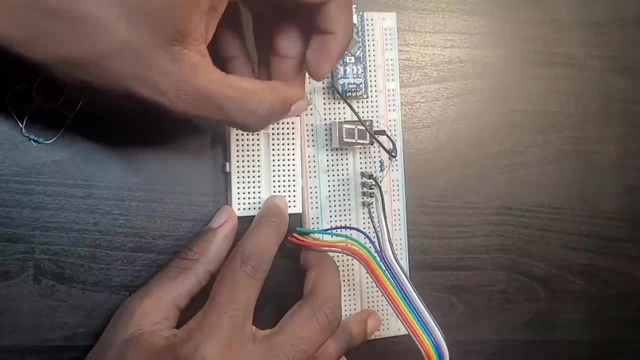 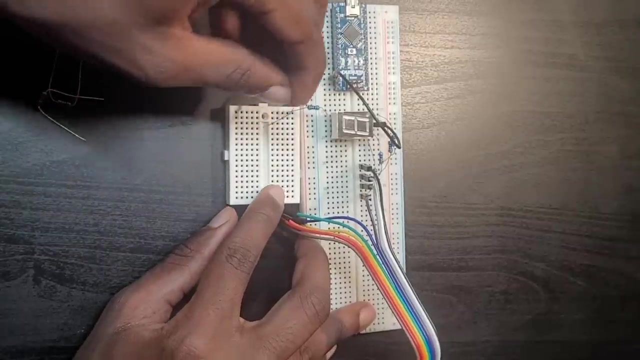 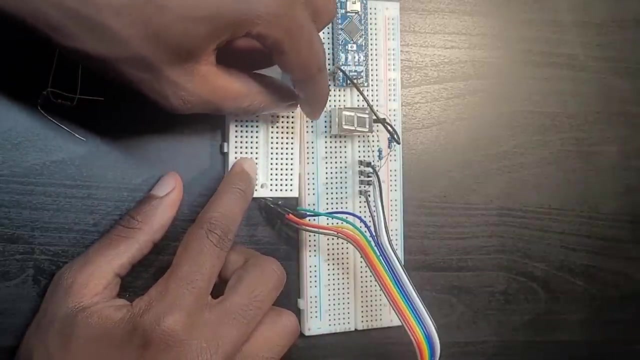 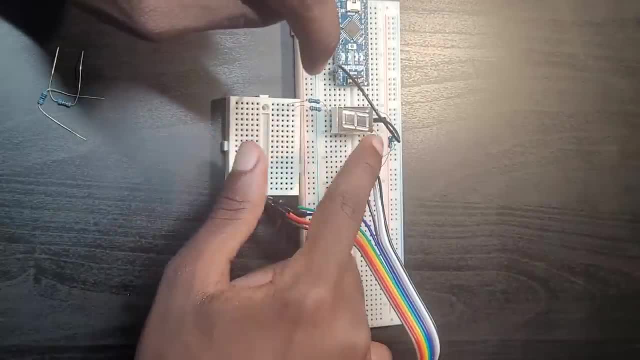 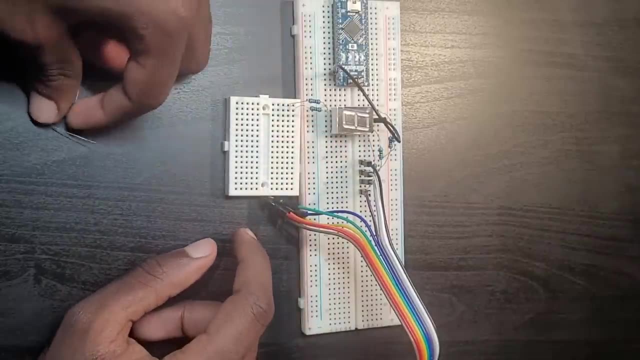 of the common pins. So, as I said again, we have two common pins and we have two common pins, but we're going to be using only one. Okay, So you either can use this one or you either can use this one. 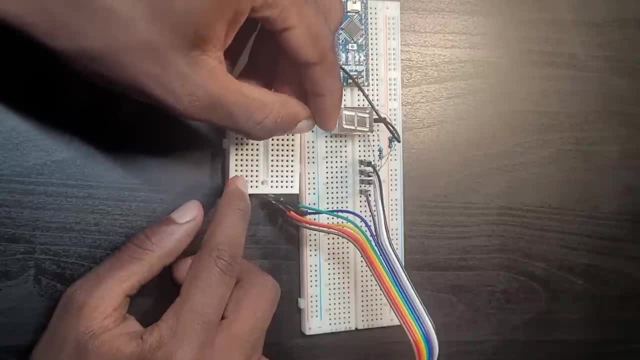 You don't use both of them, So right here, I'm going to skip it. I'm not going to touch any of it. okay, I already connected the GND from this side, so I don't need to connect it from this side. 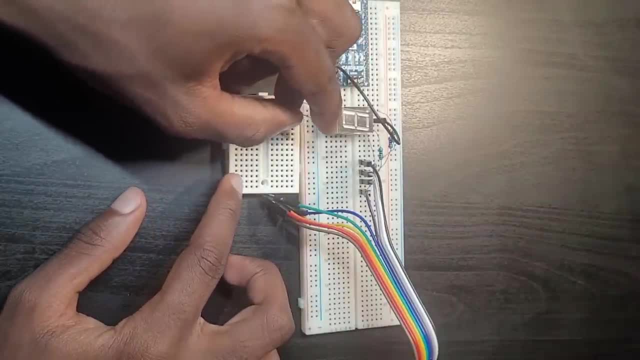 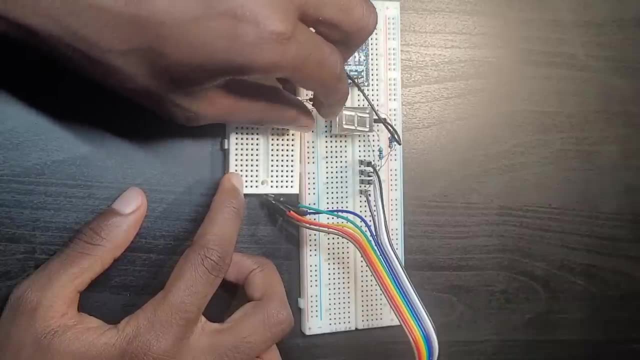 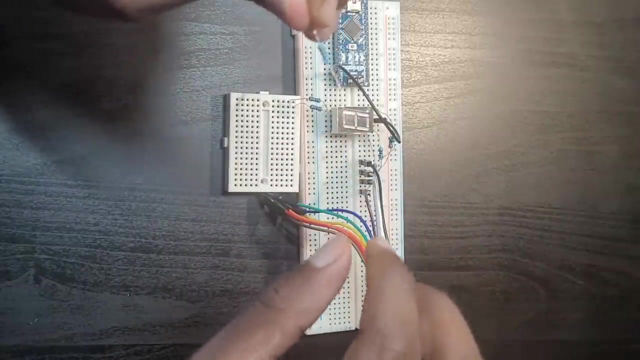 So the third pin is going to be skipped, totally okay. Now I'm going to go to the fourth one, the fourth line, right here. I have to push it a bit. They're a bit hard resistors to put in. Let me first just straighten it out myself, okay. 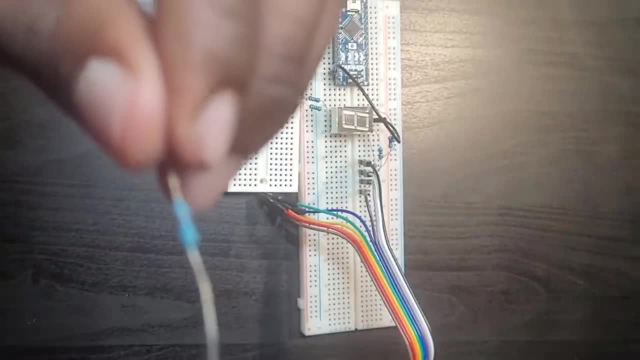 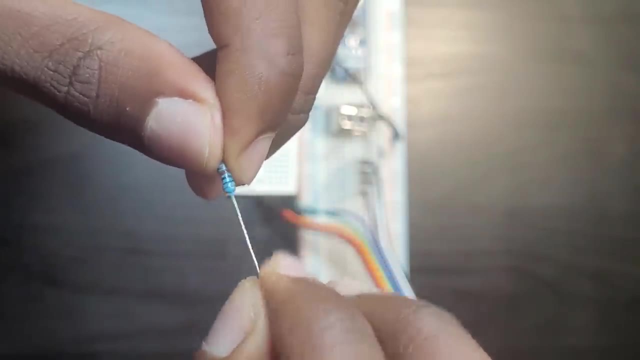 Just make it straight. Let me focus on the resistor for now. Let me bring it closer and actually focus on the resistor. There we go. Now, what I'm going to do is straighten it out. Once I'm done straightening it out, I'm just going to do is bend it. 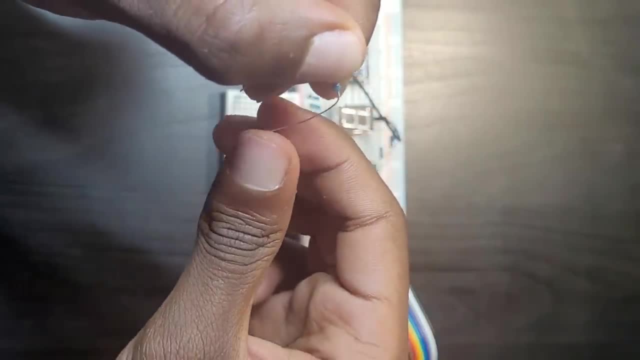 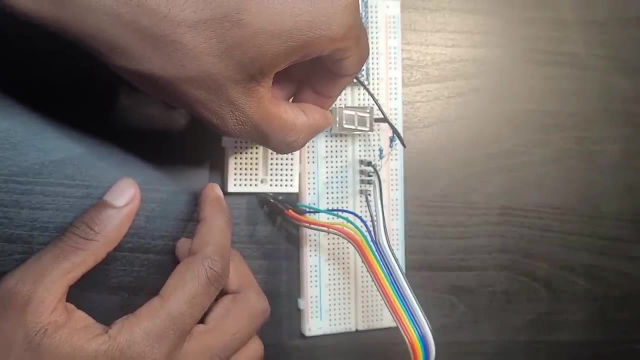 Okay, there we go. Bend it. There we go. Now let's focus on putting it back in Because, as I said again, the resistors, they do not fit in properly. Sometimes it can be a big of a problem. 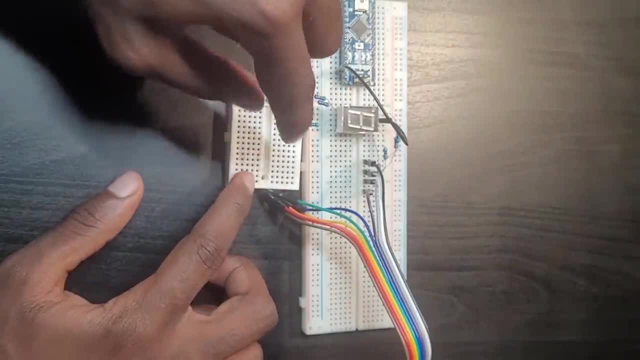 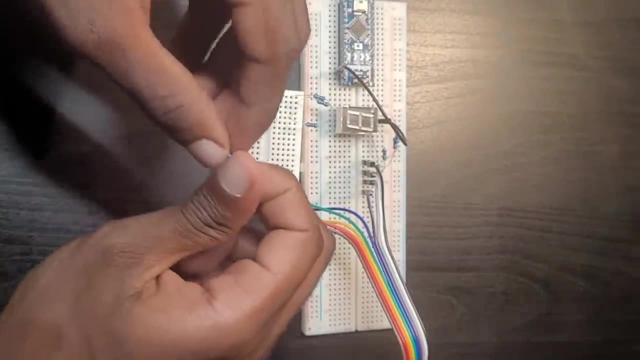 This did not fit the best. I think it's going to cause me problems, But I think it fits. Actually, I think it fits, but it might cause me problems after a bit while, So let me just bring my final resistor connect it. 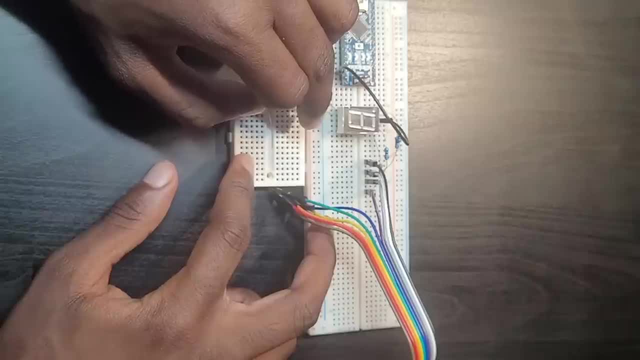 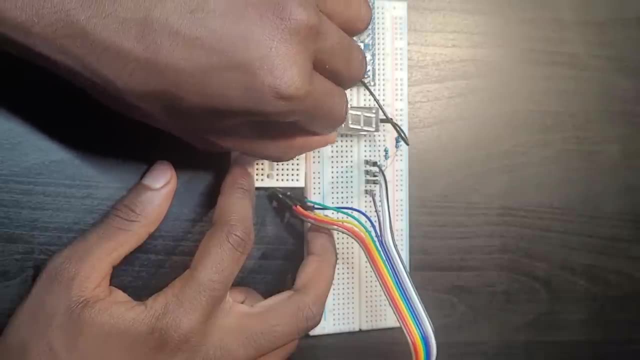 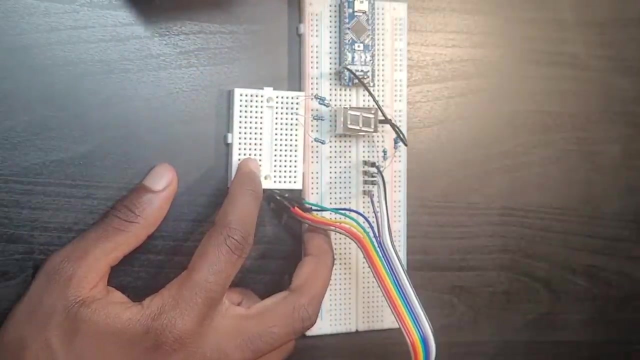 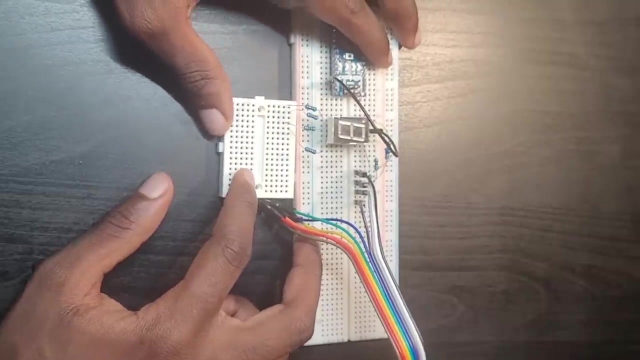 Okay, Okay, I'm going to connect the fifth one. I'm going to connect the fifth pin to the fifth pin. There we go. Can you see it? I connect the fifth one. I cannot pick it up, as I said again, because the resistors are going to fall apart. 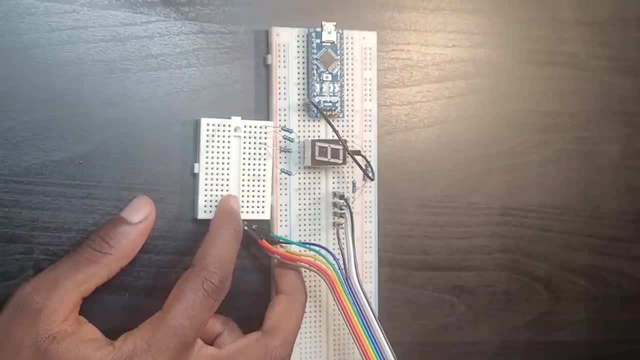 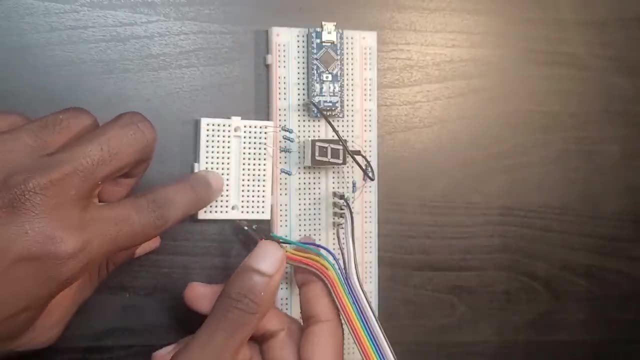 I'm just going to move it very, very slowly to the middle so you guys can see the frame. All right, there we go. Just need to be very careful with it. Okay, Now I'm going to be connecting just blue wires. 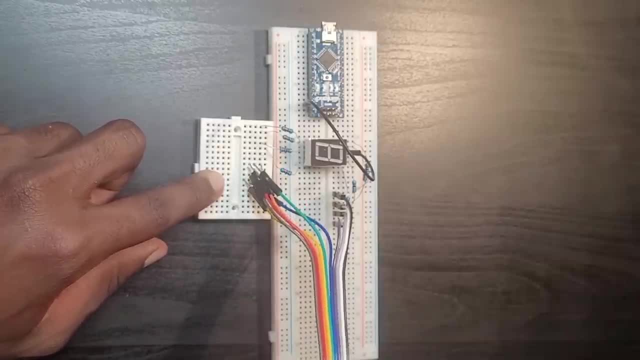 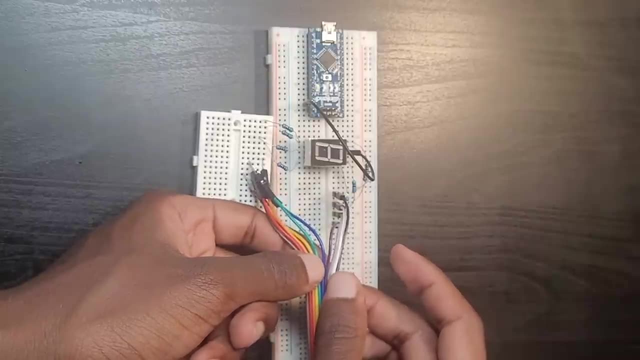 As you can see, I don't know, I don't have enough, what enough length to go here. So what I'm going to do is just going to move this totally. So what I'm going to do is from purple to blue. there's what there's a difference in. 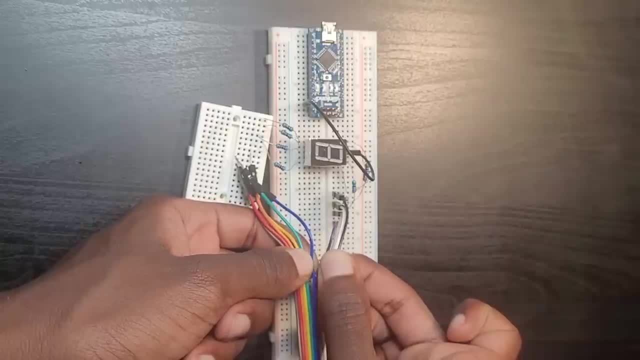 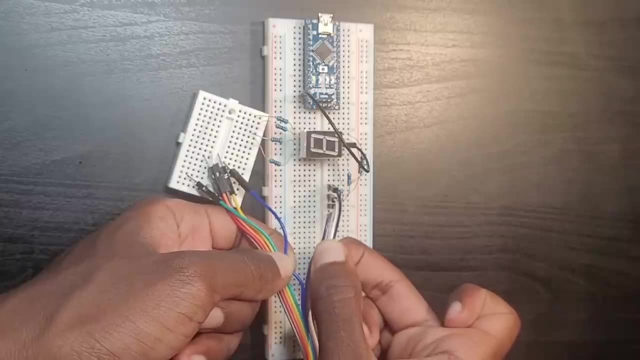 So I have to change my direction. So what I'm going to do is wrap it more. Can you see this? I'm just going to separate it. It can be separated. There we go Slowly. Can you see me? I'm separating it. 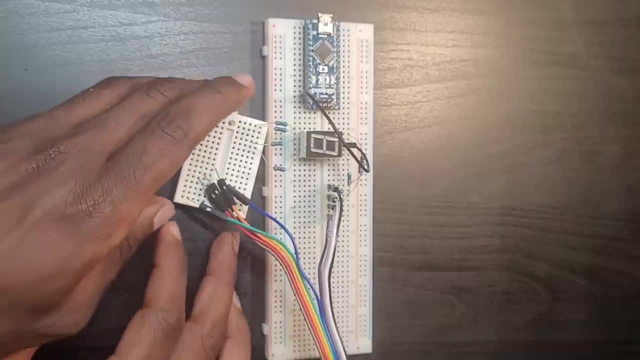 I don't want to separate it completely. If I do that then it's going to be useless. There we go, So that it has more space. I want to move it A bit of the resistor, So I don't want them to move that much. 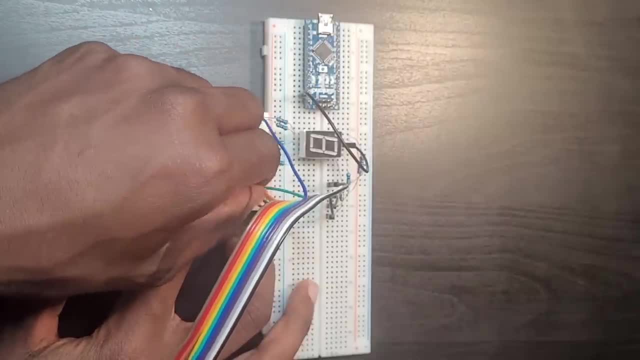 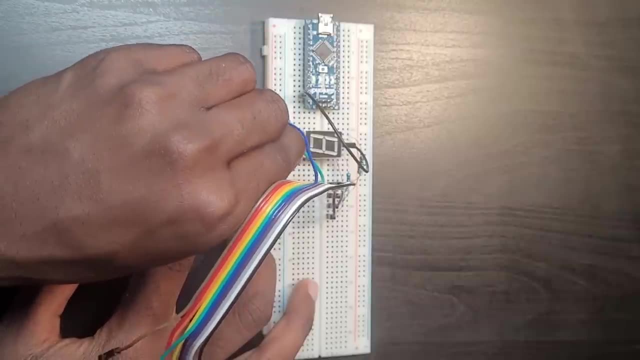 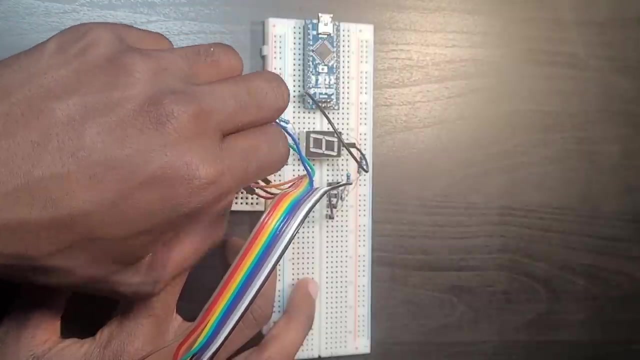 There we go. We got our first, Then we need our second. What comes after blue Green? All right, Let's use the green. There we go. So third one is going to be orange, Or actually yellow. Yellow is. 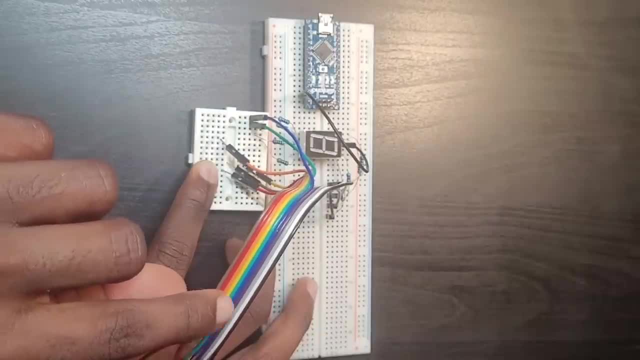 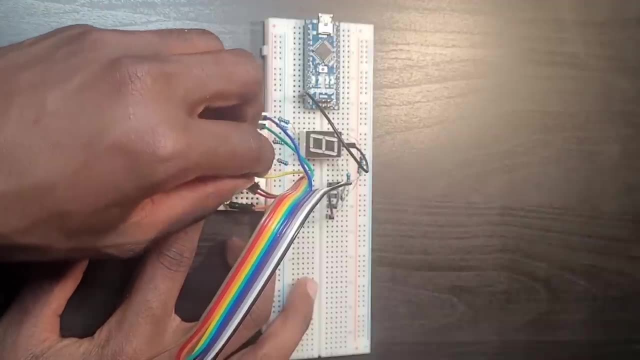 The next one, not orange. I can see it for the. I can see the colors from here, So it has to be after green has to be orange. It's our yellow, So I'm going to bring yellow, not orange. See that. 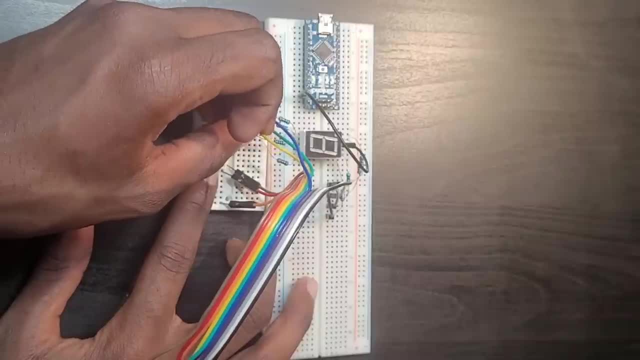 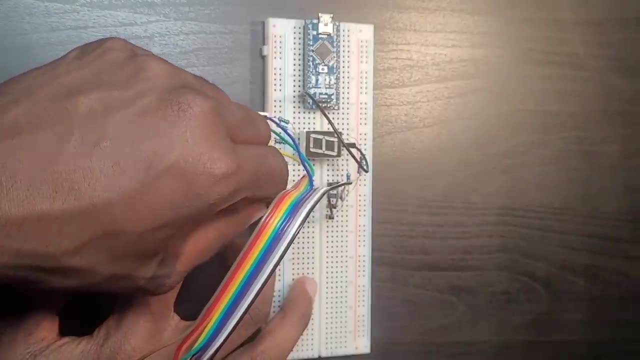 Well, that's why it's very useful. It helps me again. Okay, I'm going to skip the third pin and go to the fourth one. It's very useful because I can just reference it from here. They're attached, So I'm using a lot of pins. 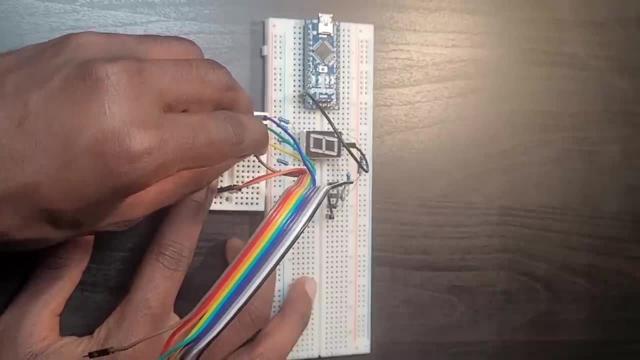 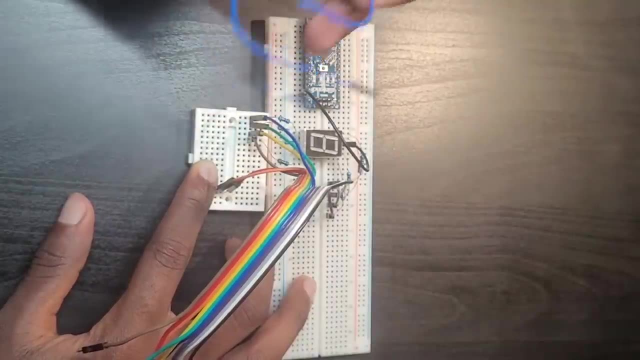 I can, just when they're, when they're put next to each other. I can use this type of wires because they make wiring way much easier, Because if I just wired them with this normal again wires, I'm going to come back here, check everything, track back. 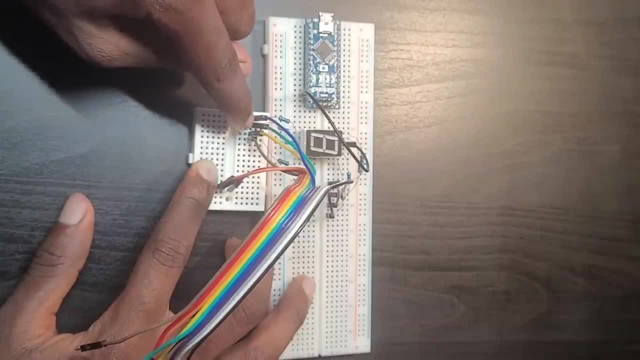 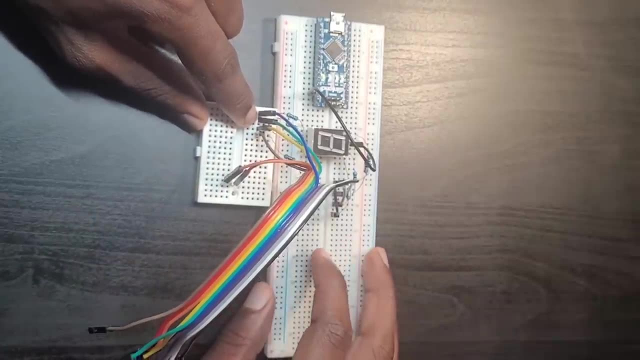 everything like this, and then see where they're connected And it's going to be a bit of a hustle. Okay, So I connected these four, I skipped the third one and I connected the fourth, Right, Good, I don't want to move it too much. 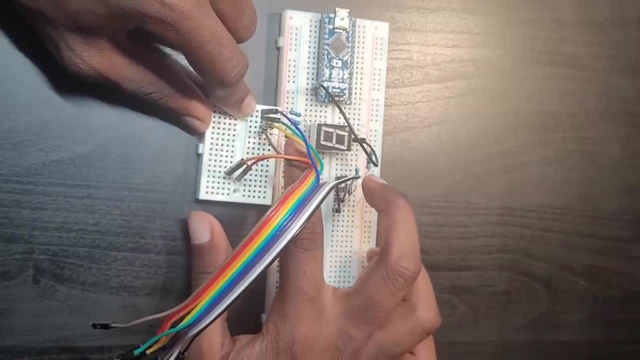 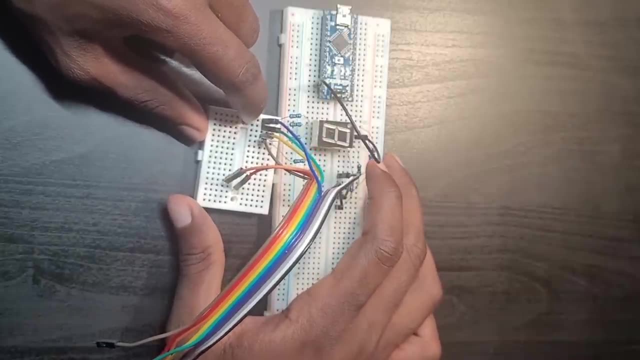 It's moving a lot. I don't like that, Not a big fan of it Moving The resistor stones seem to be holding. I'm holding them in place because they're weak. Wait, it seems to be moving a lot, Okay. 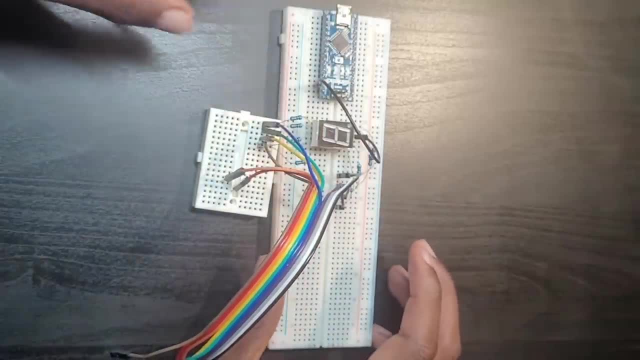 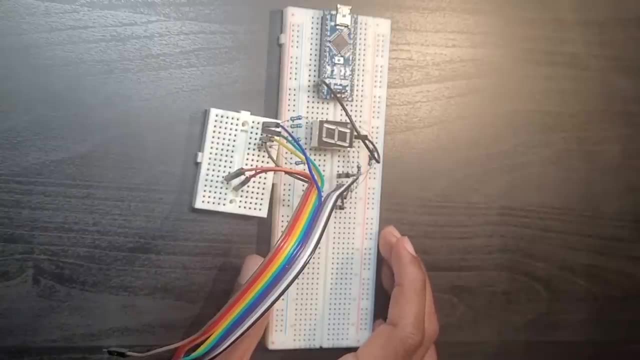 So what I'm going to do is separate the wires again. I think the wires are just having a lot of tension on them, but actually I can keep it like this, to be honest, because, yeah, I can keep it like this If everything is intact. let me just check it. 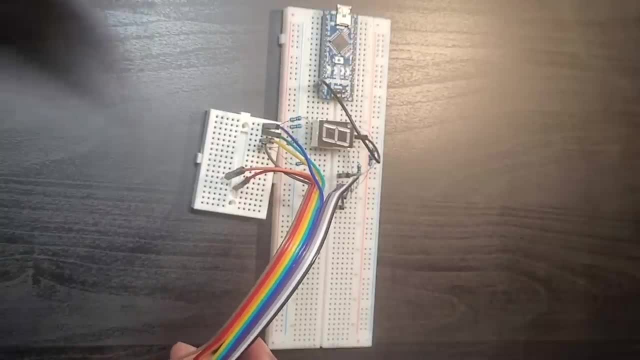 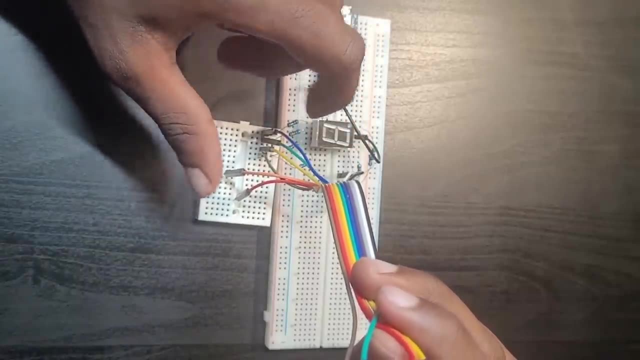 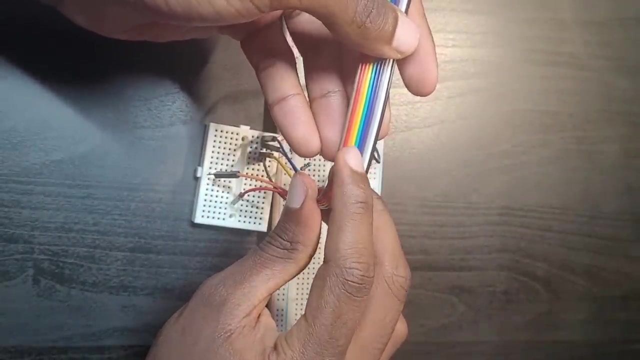 Everything seems to be intact, So I can keep it like this. actually, besides, just need to be careful when I move the wires. again, when I flip this, we'll just slowly flip it. Ooh, it's moving a lot. I'm just going to try to flip it. 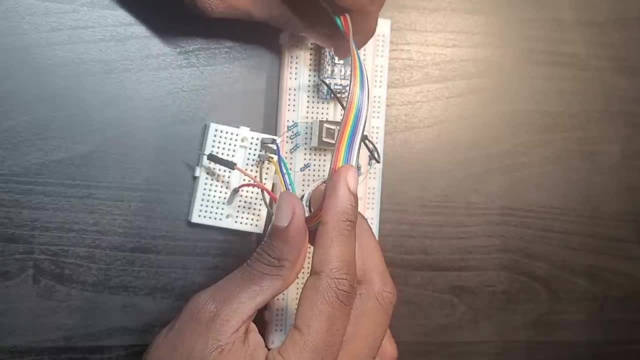 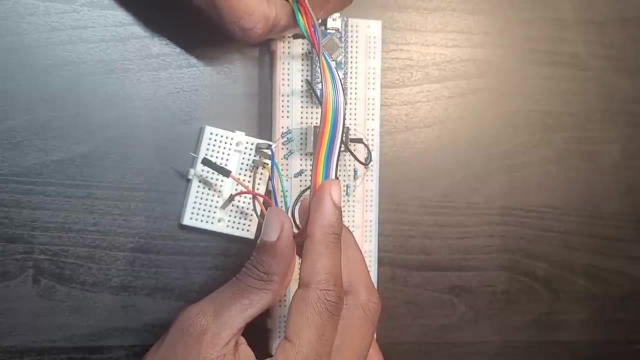 All right, Let me just connect it to some random pin so that it holds together. I'm going to come back and solve this. I'm just going to connect it into some random pins again. Obviously, don't turn your Arduino while you're doing this. 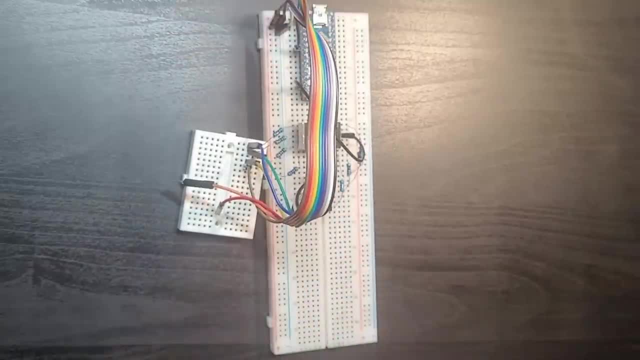 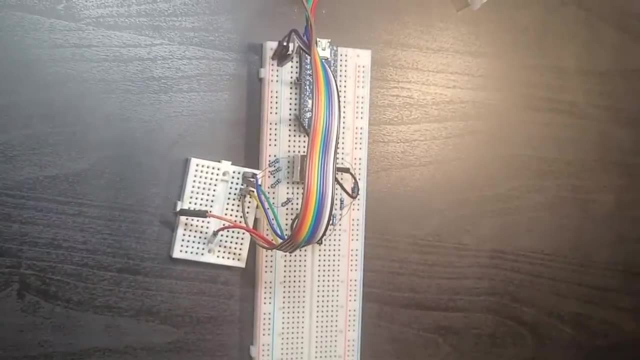 It's dangerous. I can just short the circuit right here. I just connected it so that again it just moves. Okay, I just connected it randomly. All right, Just make sure that your Arduino is not turned on when you do that. 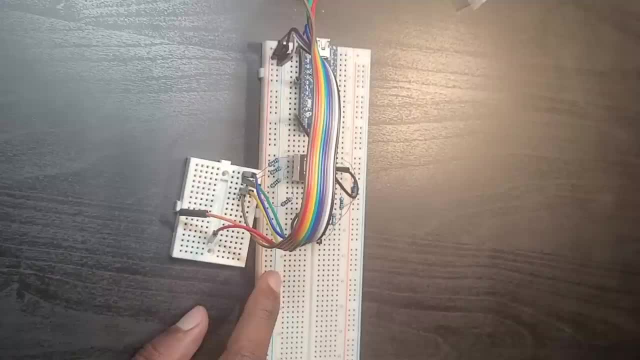 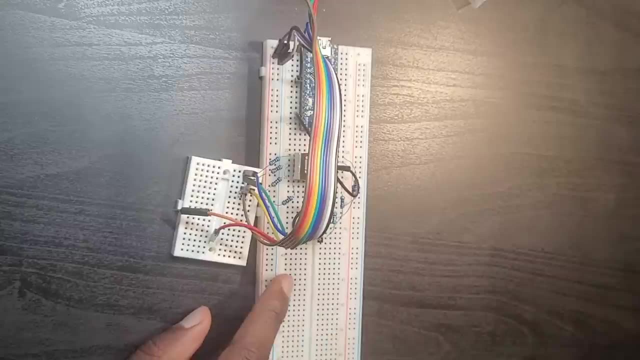 Okay. So right here, let me just think of the pins that I'm going to be using. I'm going to be using digital pins. Okay, Because I said again, I'm going to be using digital right. right here, I'm going to be using digital right. 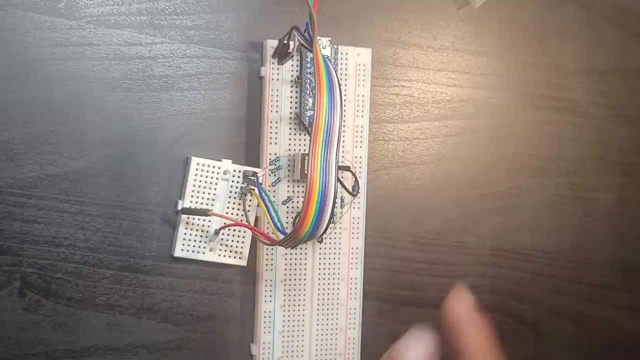 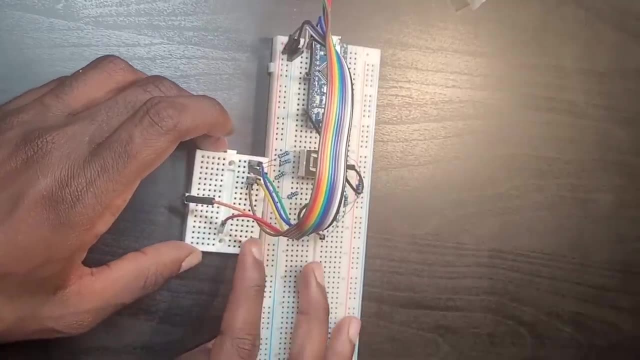 So I'm going to be using digital pins, So I'm going to need to use this side. Sorry, This is where my digital pins are, So I'm going to be using the digital pins. So, again, slowly, It doesn't. 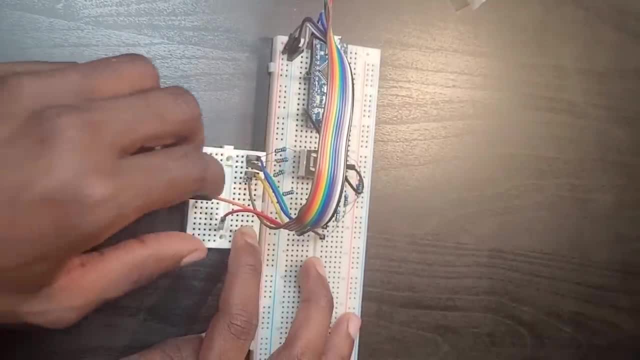 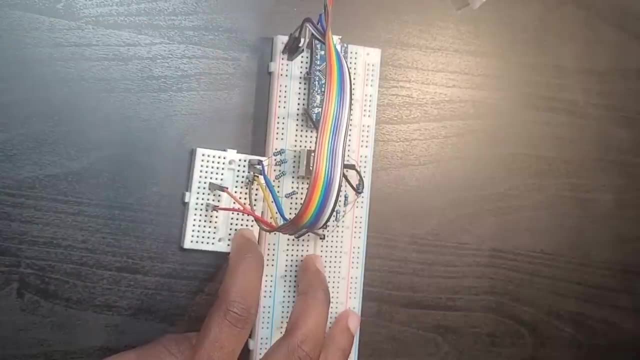 It doesn't seem to be holding the best. Wait, wait. let me just put these right here so that it doesn't move a lot. I'm not going to be using them, but again, just so that it doesn't move a lot and holds it in place. 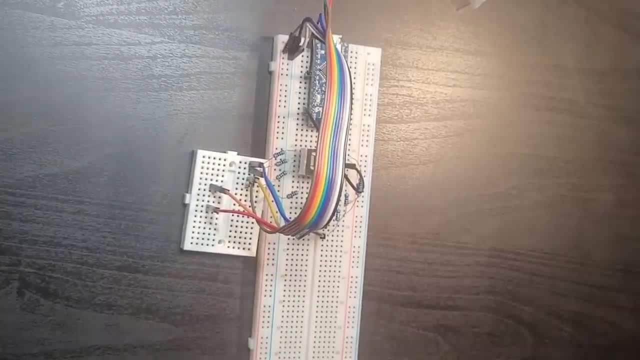 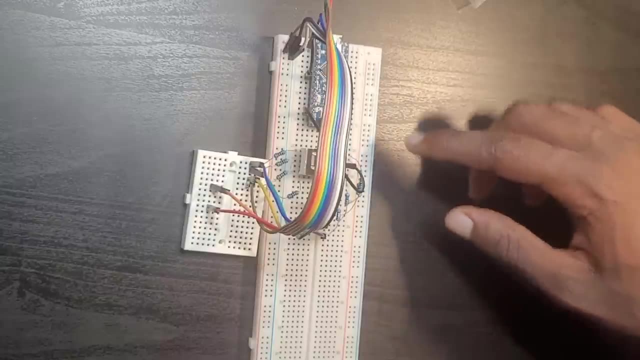 Okay, There we go, All right, So let me go over to the other side. It's a bit of a hustle. Let's go over to the other side and now try to use these pins. So I connected what Purple pins? 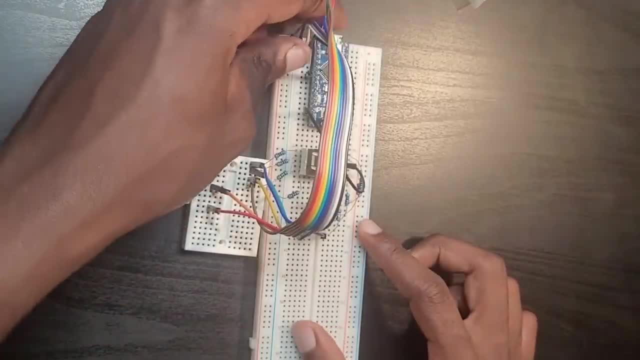 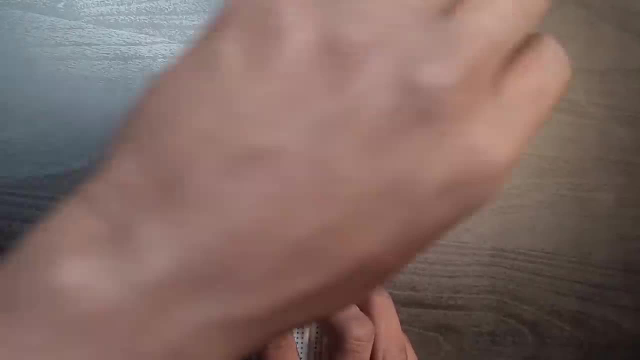 I need to get my purple pin first. purple pins, black pins, all of these that are here, I need to first them up. hold this together, Okay. So let me start with the black pin. I'm just going to start from digital pin three. 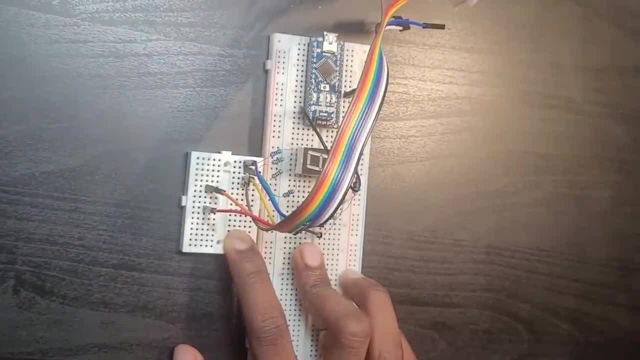 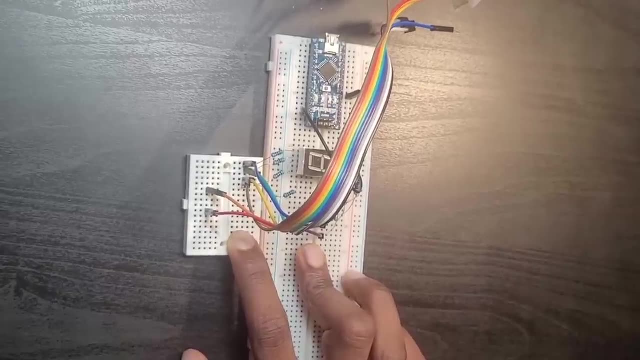 Okay, You might be wondering why I'm using digital pin three instead of digital pin one. Why not start with digital pin one, Might be wondering. Well, the thing is, there's still pin one and there's still pin zero. They're also used in binary. 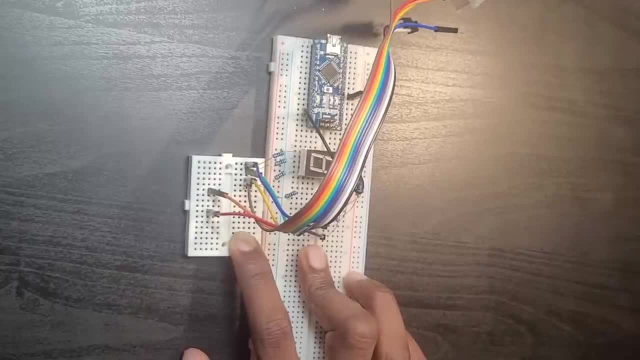 So, as most cases as possible, I try to leave them alone. Okay, I don't, I don't try to touch them as much as I can. but obviously you can use them for digital pins, but they're also used for binary. 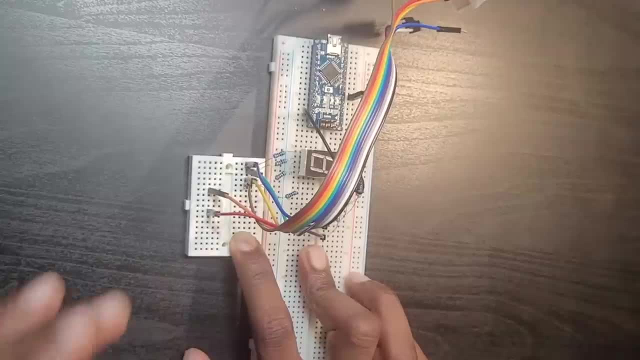 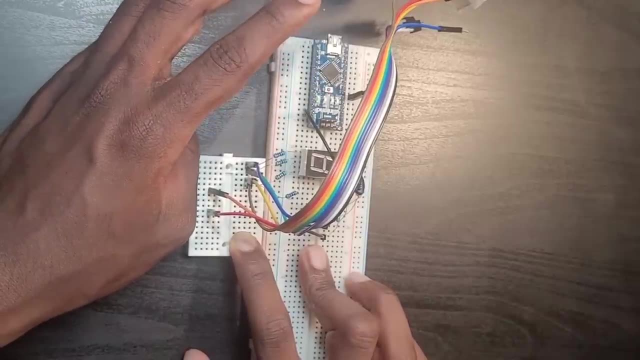 So I always again reserve them, So I just don't touch them, Okay, Because just think of me filling up digital pins, zero and one, and let's say I want to use binary. Then I'm going to have to arrange the whole thing again. 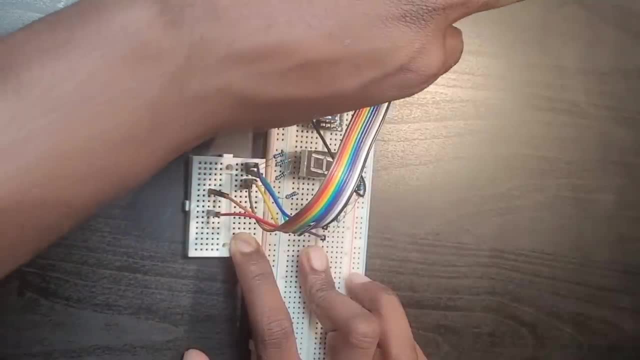 Okay, So I just leave them alone most of the time, but they work as a normal digital pin Okay. So again, you guys can actually use them. but it's just that, Again, not a practice. as much as you can. 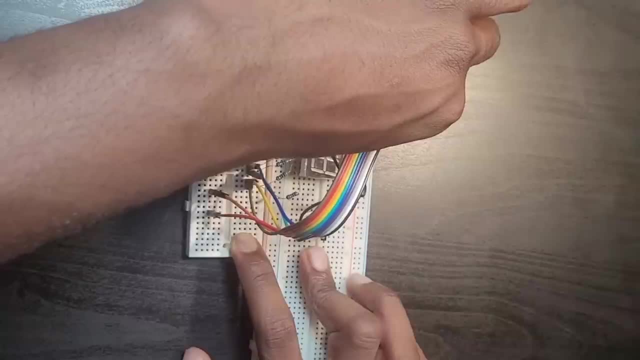 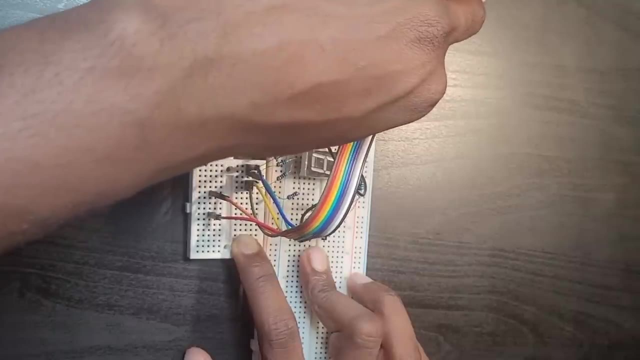 Don't use them. If you have to, though, you can use them. They're perfectly fine to be used. Let me start with digital pin two. Digital pin three. Sorry, I said there's still pin three. It is hard to even see it. 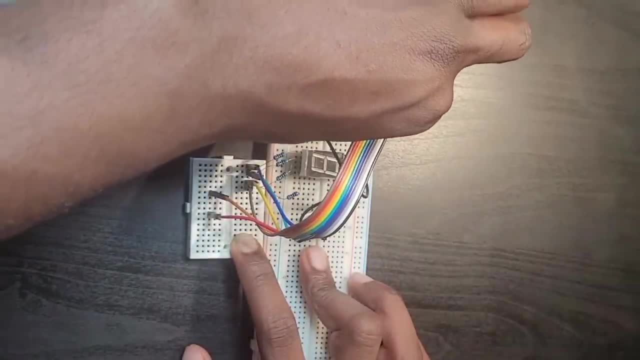 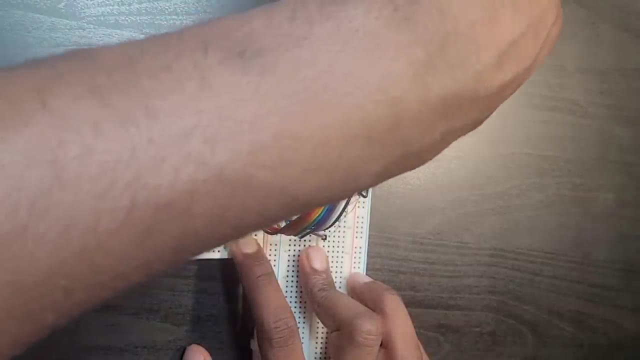 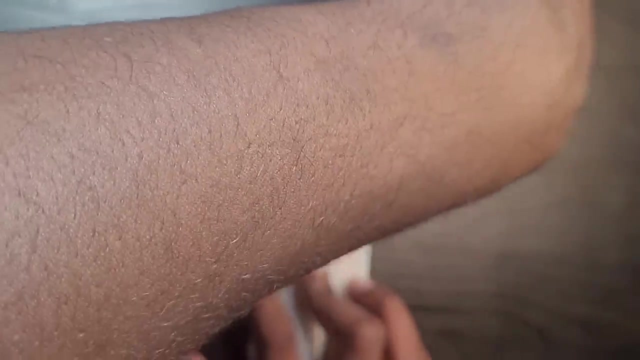 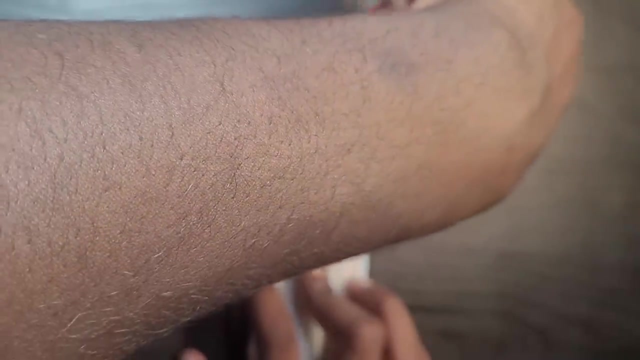 There we go After black. what comes after black? White, Digital pin four. Then what comes After white, Gray- I'm trying to get the gray- There we go. And then, after gray comes purple. There we go. Then afterwards, after, after, uh, purple, comes blue, which is right here. 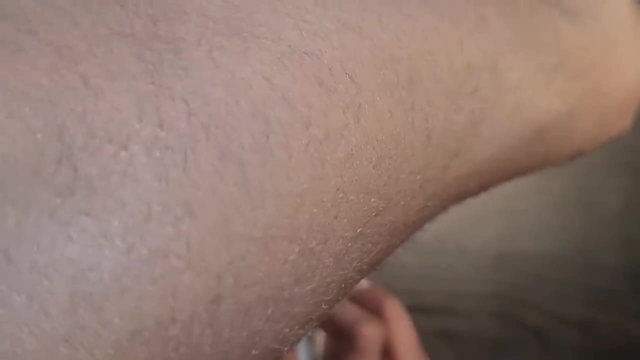 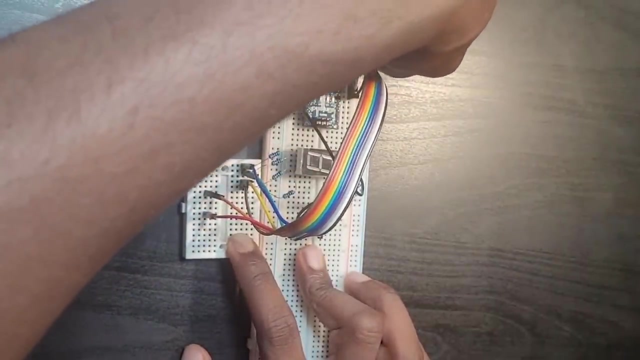 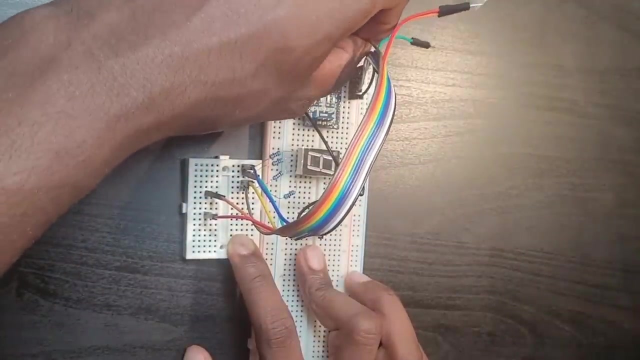 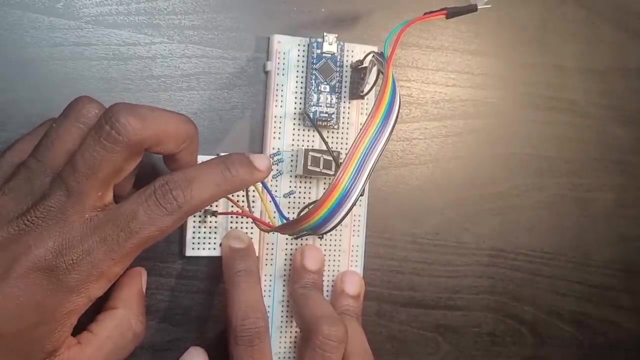 Let me go get it. Then after purple comes green. we'll just make sure that I'm not skip anything. There we go Got yellow. Then at the final one I have what I have: brown, obviously, just including the- uh, again, the GND or the common pins. 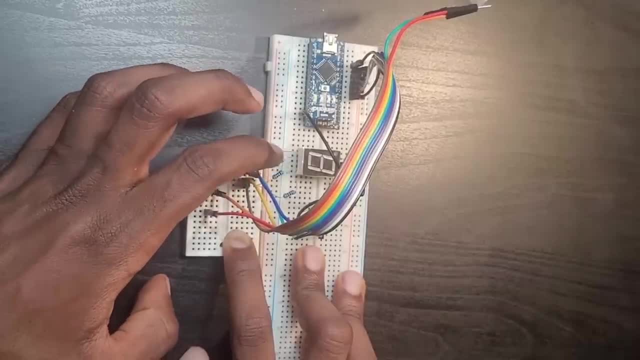 I have what pins, how many pins to connect, at 10 pins to connect And again, discarding this, disregarding two common pins, it's going to be eight pins. So let me just count this: If I'm correct, One, two, three. 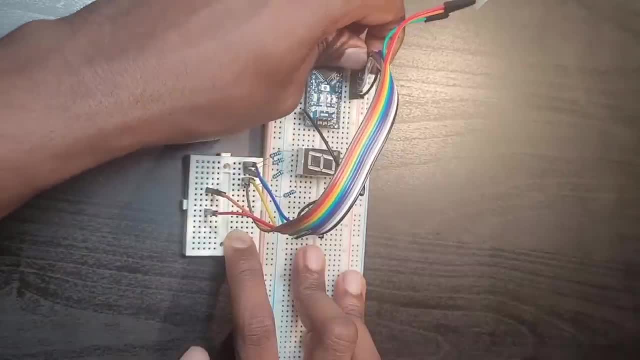 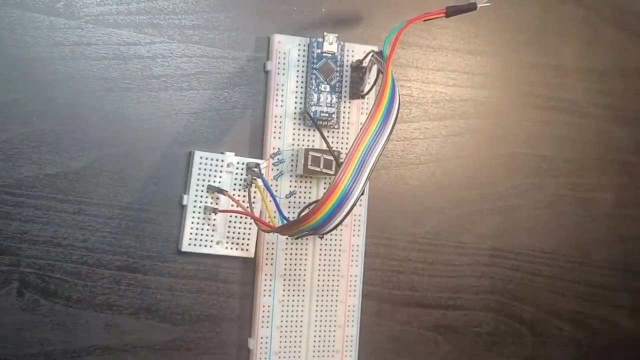 Three, four, five, six, seven, eight. So I connected eight pins. Let me just make sure the white is cut, The yellow is connected properly. There we go, And now everything is connected. Can I just need to be more careful? 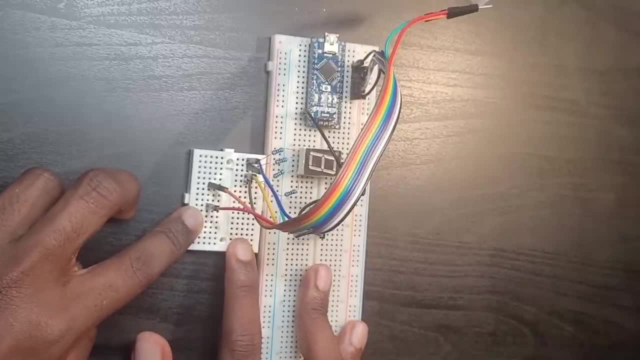 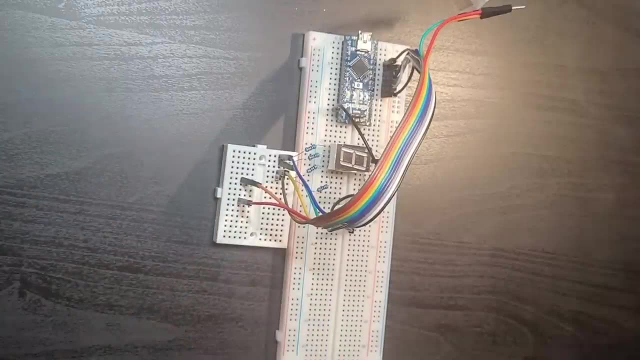 Okay, Again, I'm using these, as again, as a support. they're not connected to anything. Just keep that in mind. Don't want to move them a bit. We have to move them a bit. I'm not going to touch it afterwards. 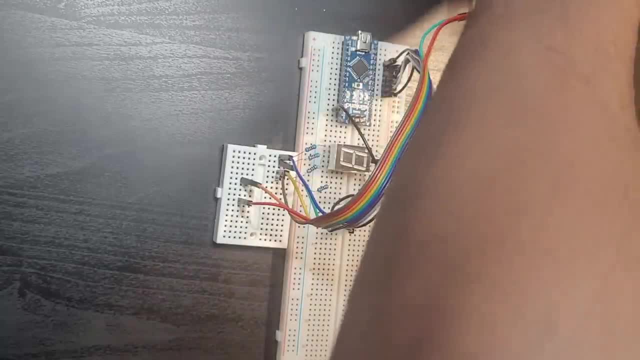 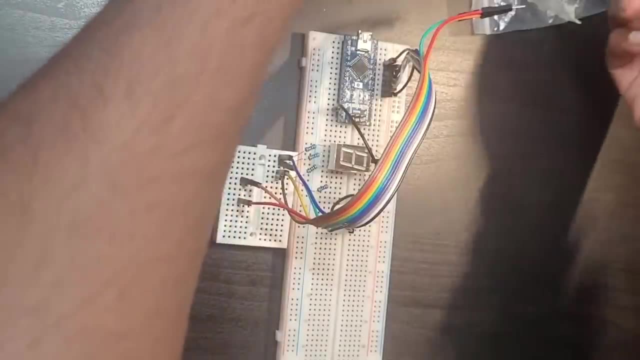 There we go. Let me just bring my Arduino wire. There we go. I'm just getting my. let me wire up my Arduino, Just bring the wire. Let me just keep it here. Okay, It was a bit of hustle too. 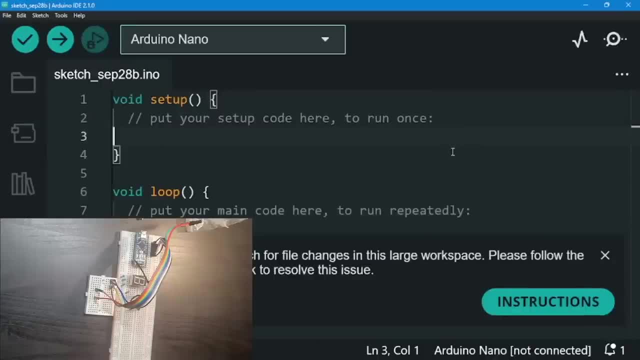 Again even connected. Okay, So now let's start writing down the pitch. Let's start giving them names. Okay, Let's begin. So go right here And give start Giving them names. Okay, So the first thing that we're going to be giving out name to is pin three. 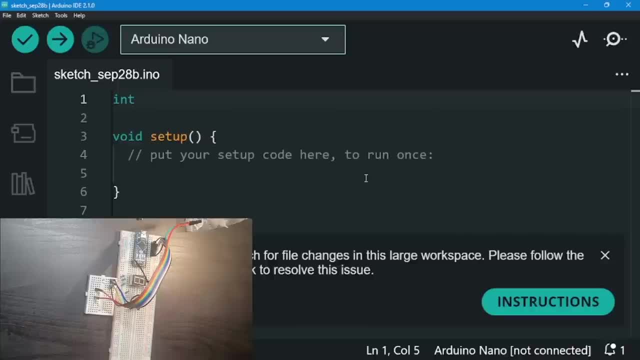 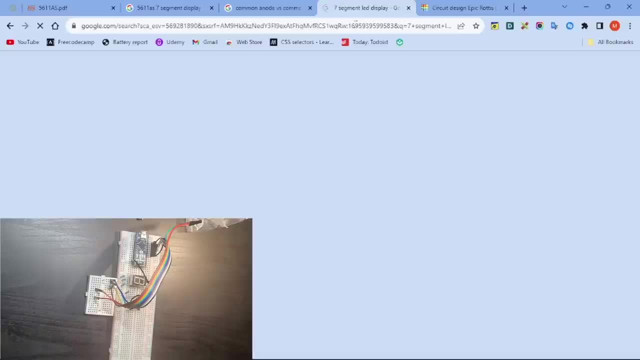 First things first, Again, we need to understand what part is going to be lighting up. Okay, So let me first I'm going to need what I'm going to need: the diagram. Let's get the diagram. I'd say seven segment led display. 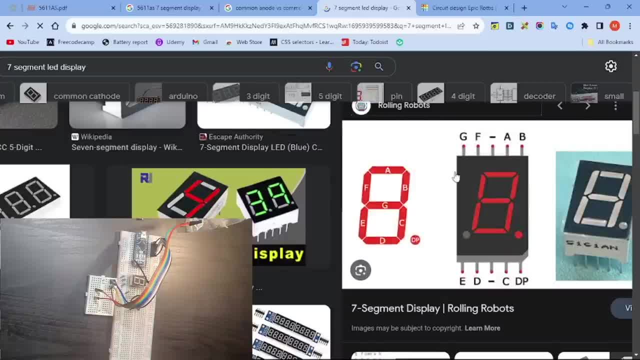 Let's go to images and find a diagram that has. there we go, We find a diagram that has what they're naming. It's going to be six. Okay, So let me start from here, the very most left from here, from this side, it's going to be: 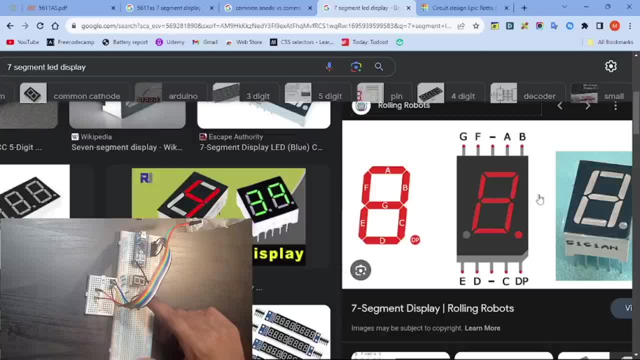 what the very most left side is, what it's going to be? the black one, the black wire. the black wire is connected to what To pin? number three, Okay, It's going to pin number three. What is it? Decimal point. 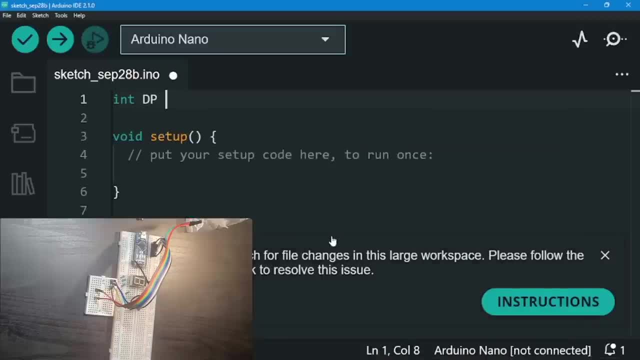 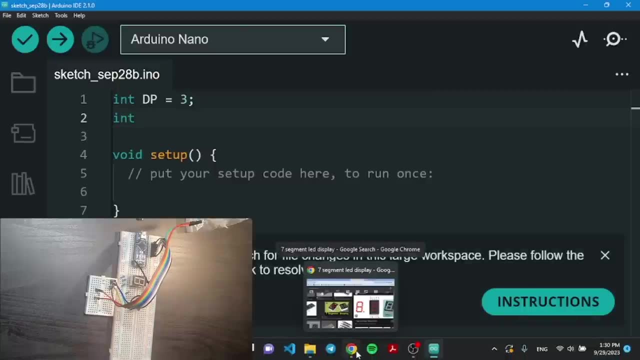 So what I'm going to say here is integer, DP, What is it? Pin number three: integer. What else is there? And keep comparing them. So what I'm going to do is actually there we go, Divide them into two, right here. 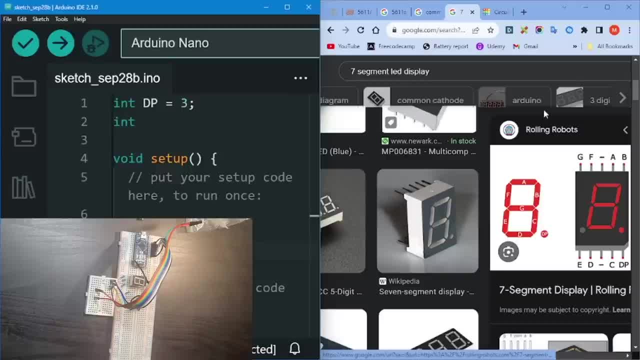 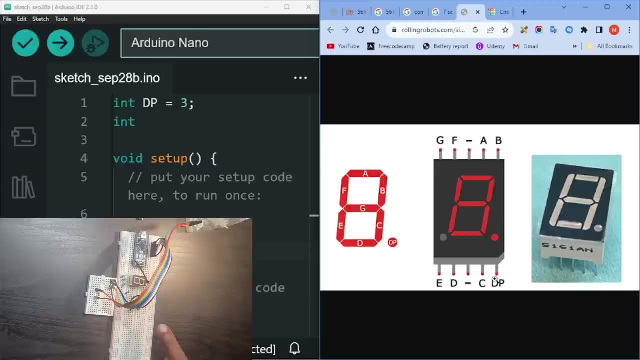 So you guys could actually see them. Let me just get the image. let me just get the image, the full image, and just open the image, open the image tab. let's get the whole image. There we go, All right. So now what I did? I connect the decimal point. 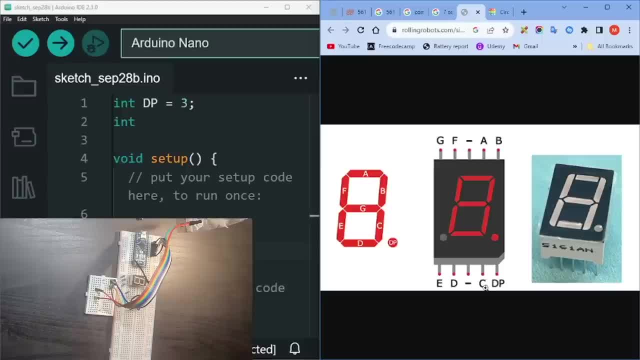 And afterwards is white Pin? white is connected to what To pin number four. What is it? It's C. So all you need to do is what C is, of course, to pin number four, that integer. again keep saying that then we skipped it. 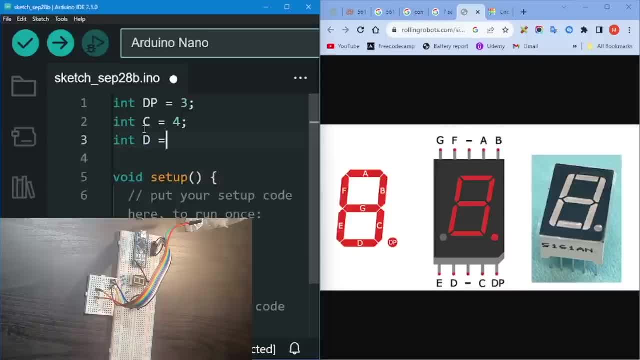 And then we went to what. We went to the silver one, which is going to be D. So D is set to what Pin five. It's going to be easy afterwards, E set to what Pin six. because they're set to what. 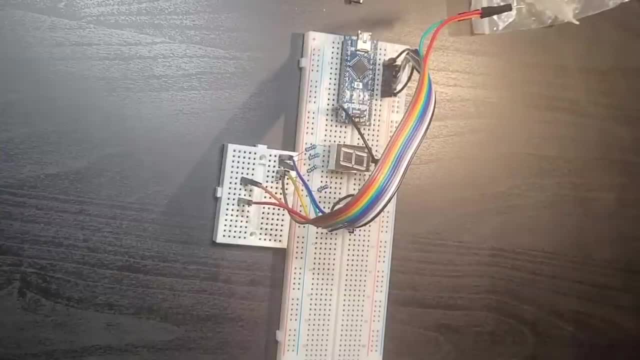 Next to each other. Okay, Then afterwards, what I need to do is: we're done with this row, I need to go to the other one, We need to go to this side, So we're going to need to check this one too. 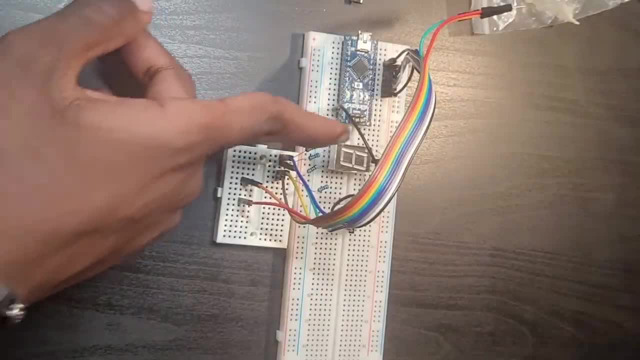 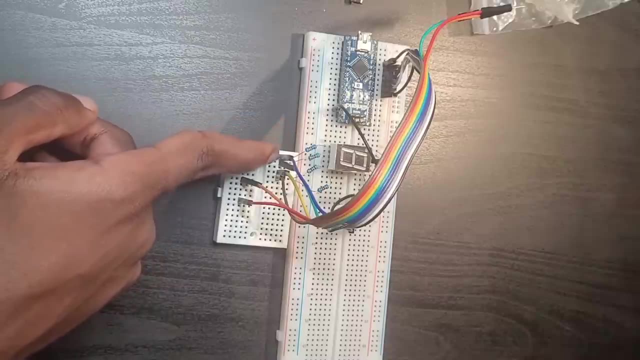 Okay, So the blue starts at the very left. The blue starts from here. As you can see, the blue starts from here. It's connected to the very left. Okay, The next after purple is what Is blue. So it's going to go. after six, it's going to be seven. 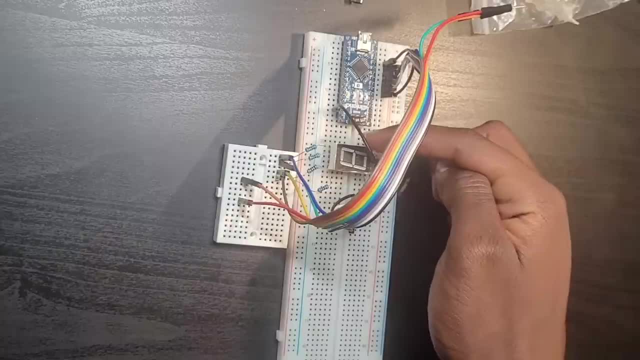 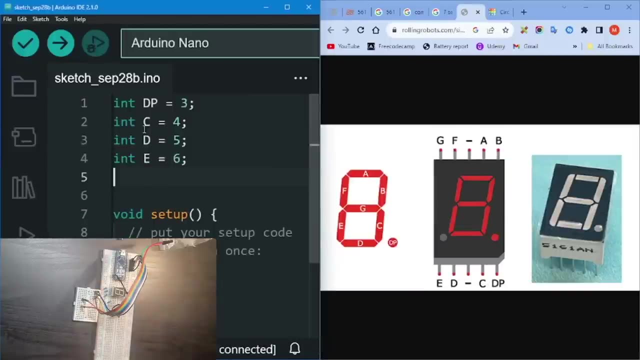 So this one is going to be seven. Okay, So the very left. again, you need to keep referencing what The decimal point is, how you're going to be referencing it. Okay, So let's look at the image. So is it going to be what? 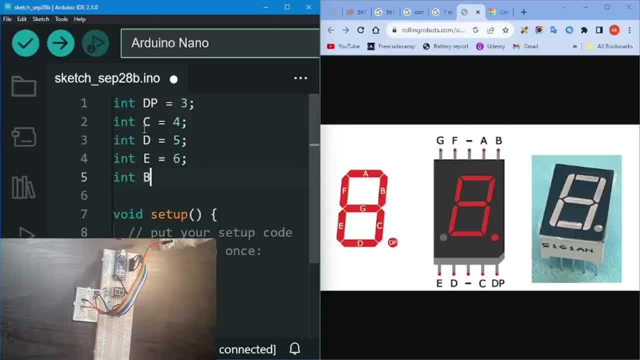 Is it going to be pin what Segment? what Segment B? It's going to be segment B. What is it set to Pin? seven? So keep going on, And then A set to what Eight, Then afterwards again, we skip the third one, the common pin. 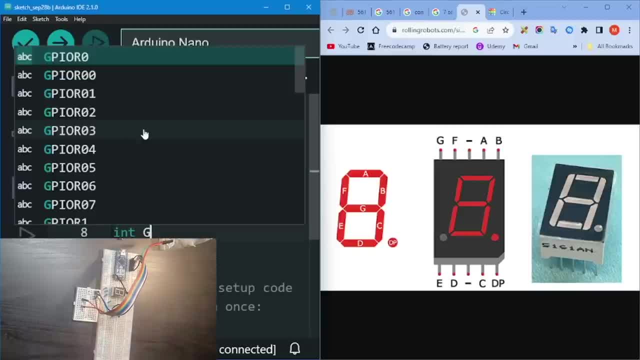 And then we go to F, which is going to be set to pin nine, And again the final one, G, set to what It's set to pin 10.. So let's even see if it ends on pin 10.. 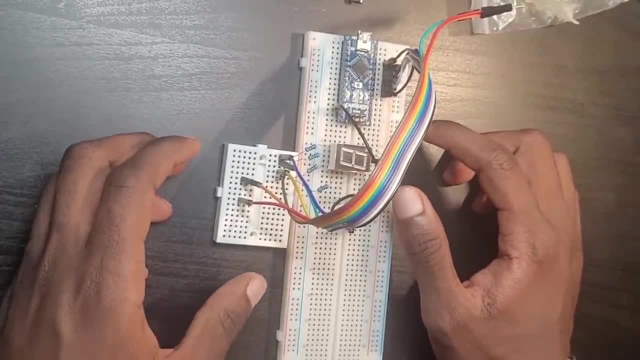 It starts at pin three. Let me just look at it. It's a bit of a hard one. If you cannot move your Arduino, it's really hard to actually look at it. Okay, we have pin 12, 11.. Okay, 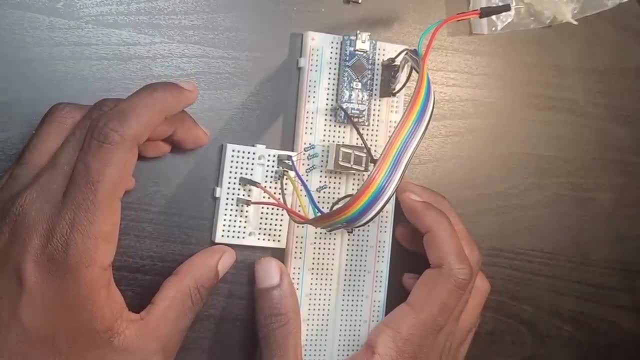 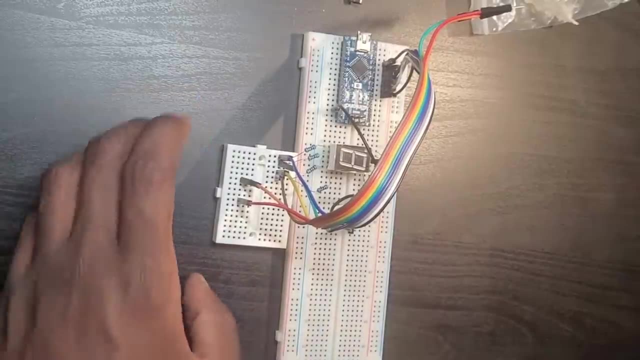 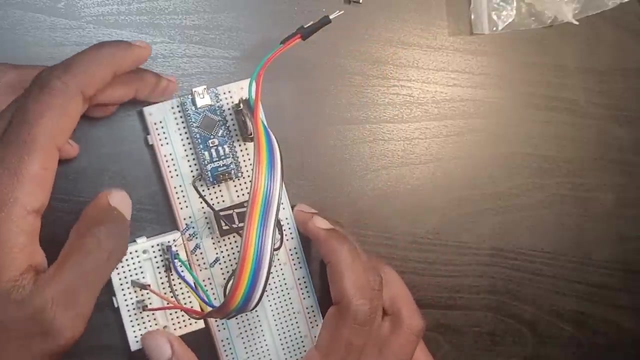 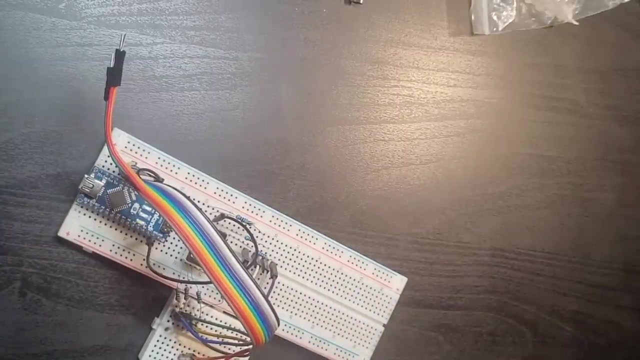 It's really hard to actually get a hold of these. Let me just look at it. So again, let's see if I made a mistake or not. Let me just move this. Let's move it slowly. Since that I stopped at pin 9, not pin 10, I might have made a mistake here. 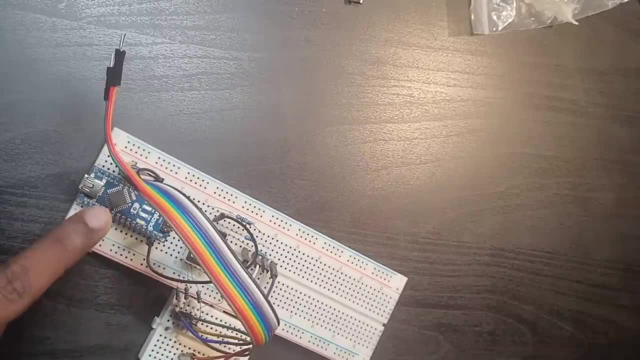 We connected 4 pins here and 4 pins here. How much should it add up to? I'm supposed to be using what? 8 pits? Okay, How many integers did I set up? 8 integers, I'm correct on this one. 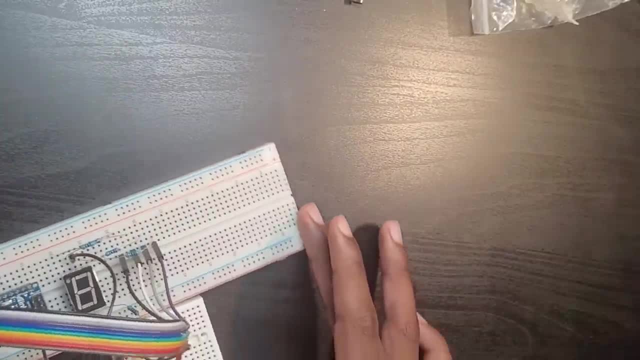 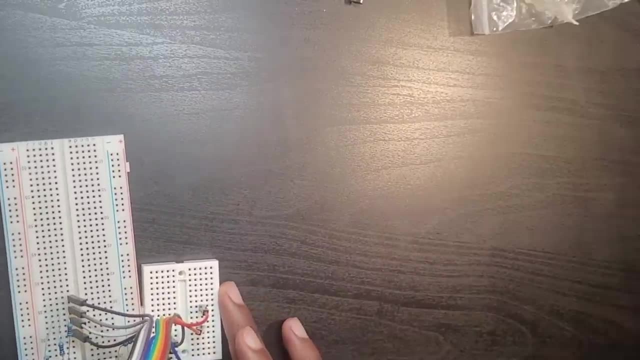 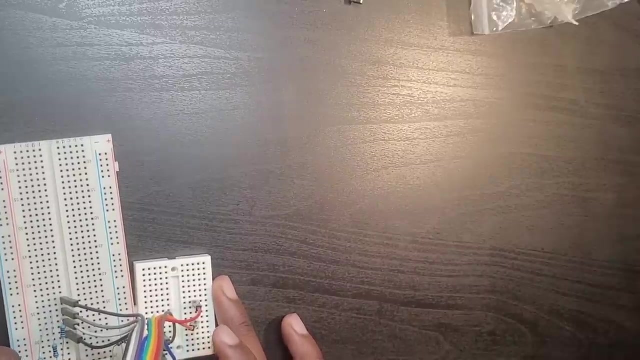 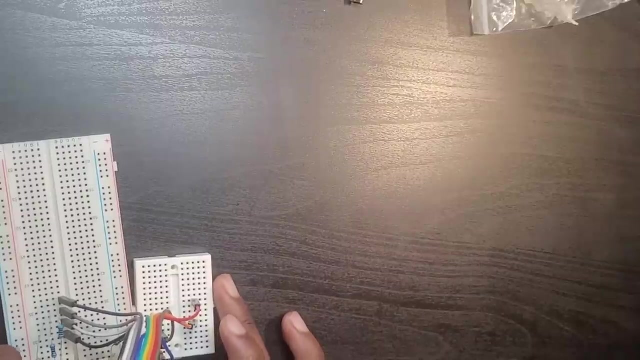 Did I start from 3 or 2?? I mean we might have started from 2.. Let me just check it. It is connected to pin. Is it connected to pin 3 or pin 2? It's connected to pin 3.. 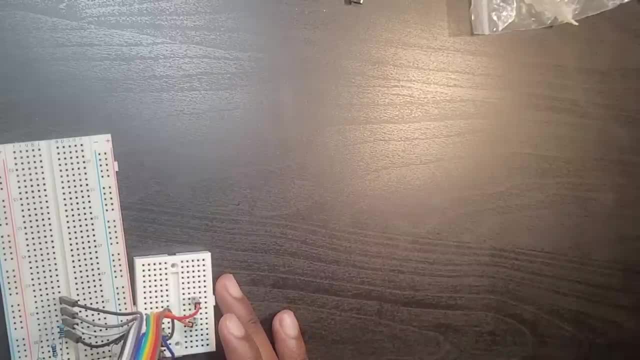 It's connected to pin 3.. I'm checking it and it's connected to pin 3, pin 4, 5,, 6,, 7,, 8,, 9, and then it doesn't seem to be connected to pin 10.. 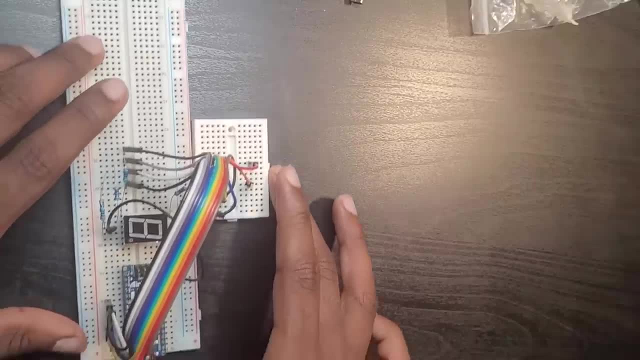 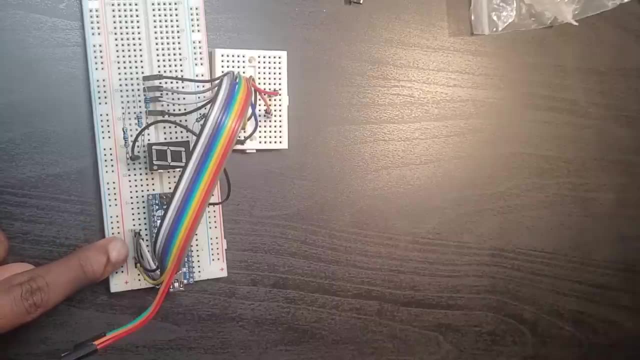 Did I forget about? Let me just check the number of pins that I connected here. Okay, I think I made a mistake right here, because it's supposed to be extending to pin 10 and it's not touching pin 10.. Let me just count the number of pins here. 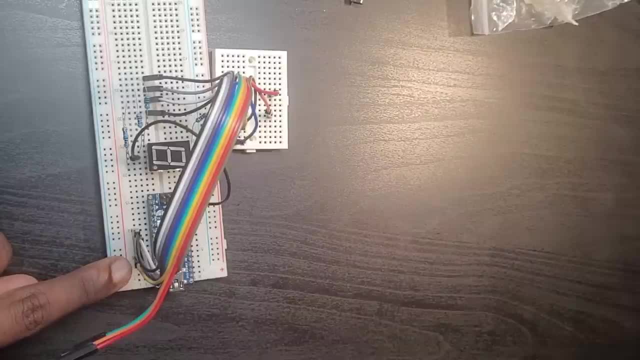 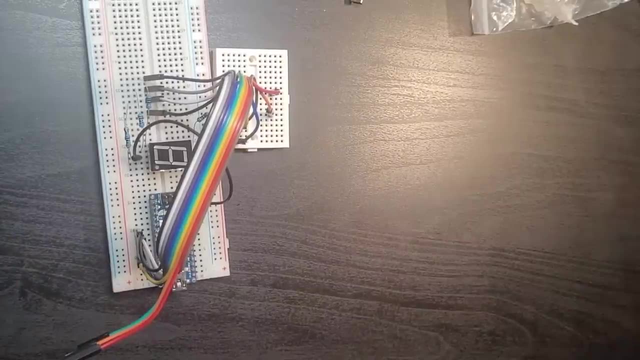 1,, 2,, 3,, 4,, 5,, 6, 7.. I'm supposed to be connecting 8 pins. I did a mistake right here. I made a mistake right here. Hmm, What could it be? 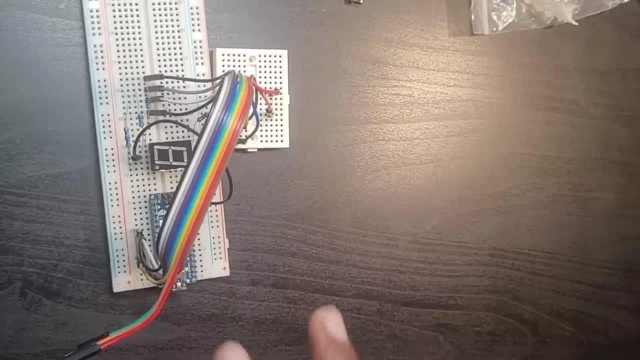 I made a simple mistake, most likely, So let me just check again. All I need to do is what, Since they're what, Since, as I said again, they're connected pins. it's going to be really easy when I make a. 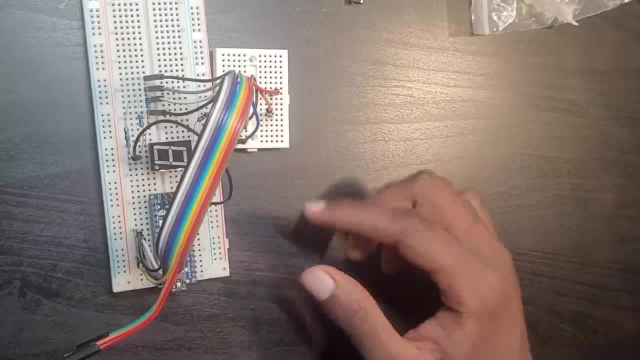 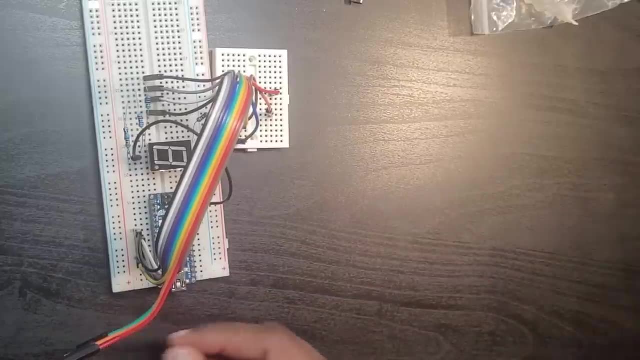 mistake. So let me just check it right here. So I connected- hmm, I did not connect the green pin, because I'm sure I connected. Okay, there we go. I connected green pin, but I did not connect green pin. So what did I do? 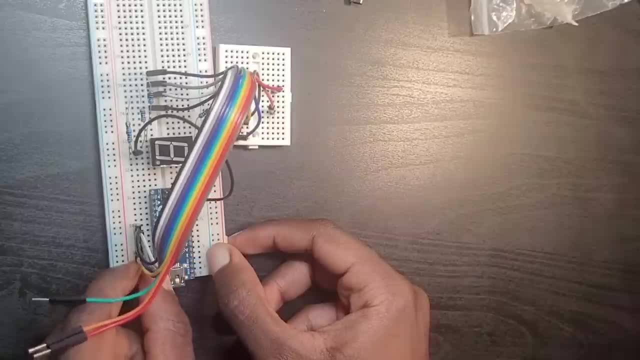 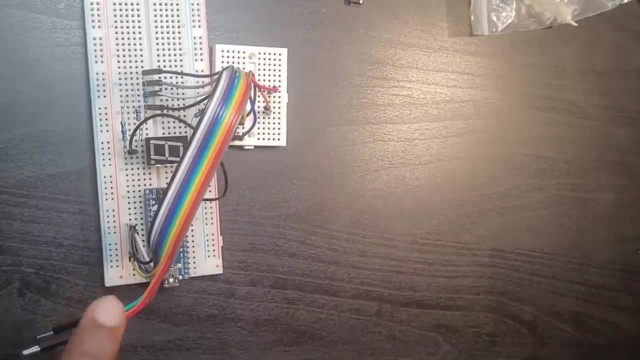 I connected brown pin here instead of green, Ooh Ooh, which is so wrong. again, Let me just. what I need to do is check it. So let me just check the colors. I connected black and then white and then gray, which makes sense. 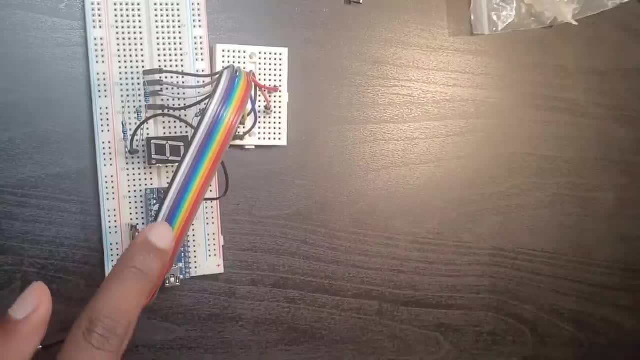 And then purple, if I'm correct, There we go Connected: purple and then blue and then yellow, blue and then yellow, But I forgot about green in the middle. right here, I'm not going to, I'm not supposed to be what. 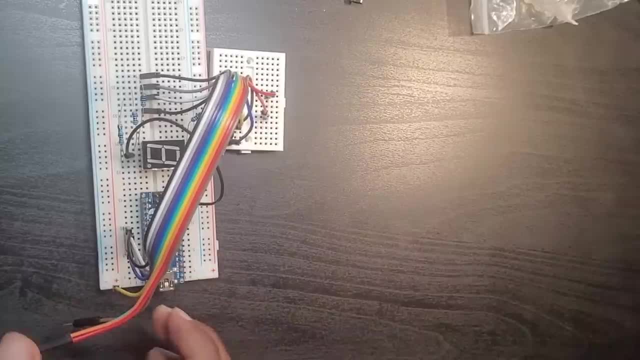 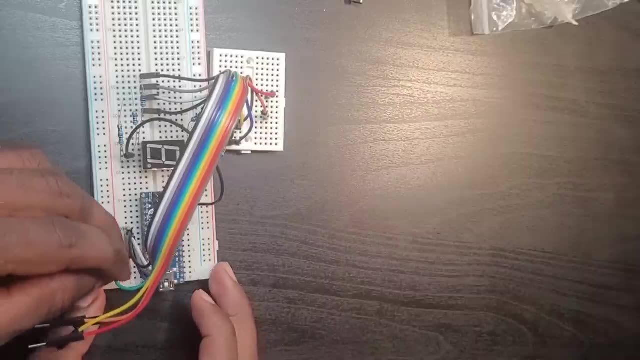 Connecting green right here. I'm supposed to be connecting green, not yellow. Ooh, I made a mistake right here. That happens. Let me just try to solve it. There we go. I made a simple mistake, but it was easy to solve. 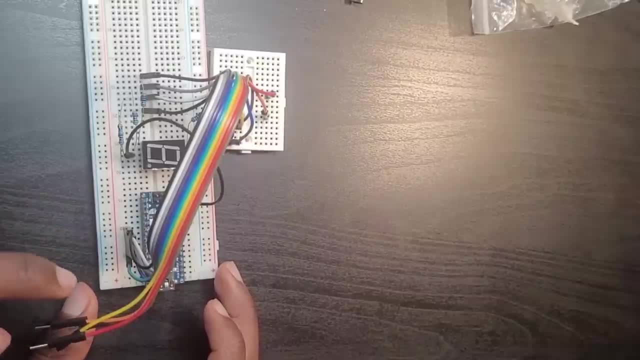 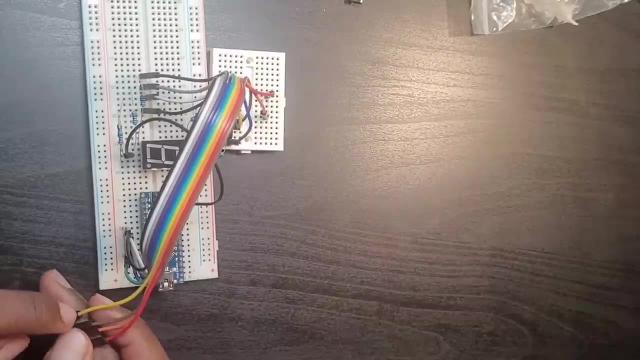 Why is that so? I'm using attached pins. That's why they're very, very important. As things get complicated, it's going to be really, really hard to fix them. It would have taken me at least 10 minutes to even find the problem if I was using normal pins. 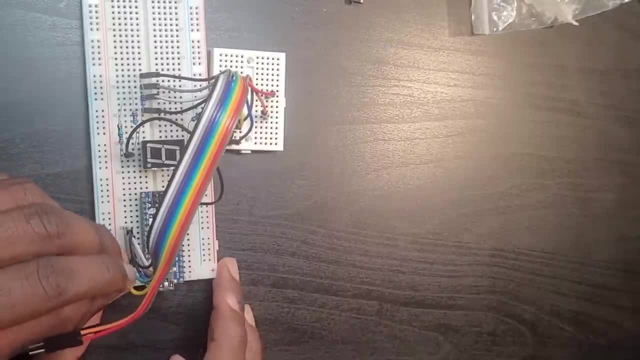 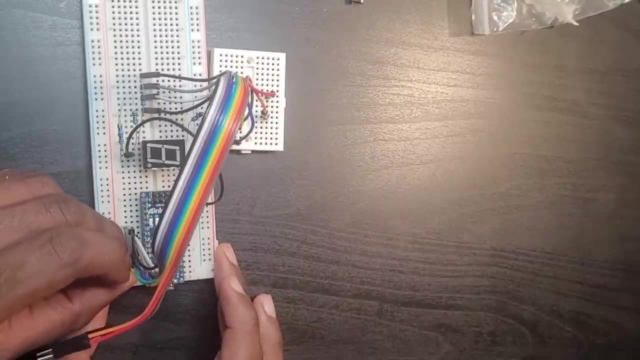 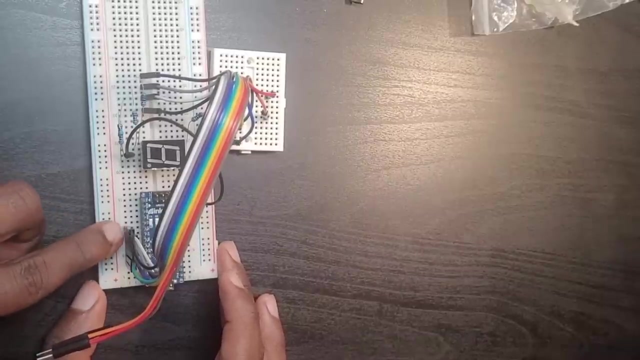 But with just using these pins, I just made it really really easy, Okay. And then what? After green comes yellow. Now am I correct again? Did I make another mistake? Okay, Now it's connected. what? How many pins? 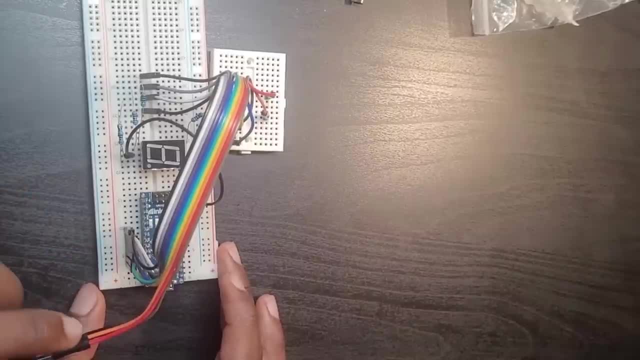 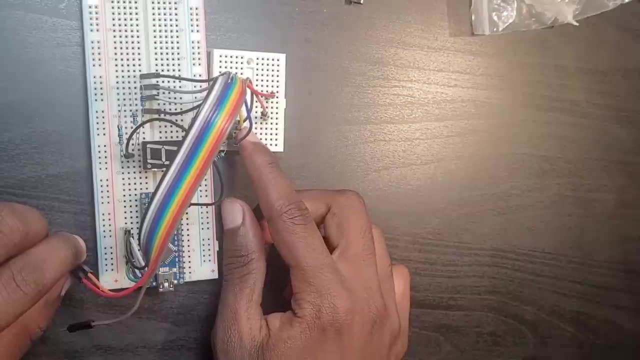 One, two, three, four, five, six, seven, And then I have an orange pin. Did I connect an orange pin here? Yes, I did, But I connected it to what? Ooh, Instead of connecting this one. 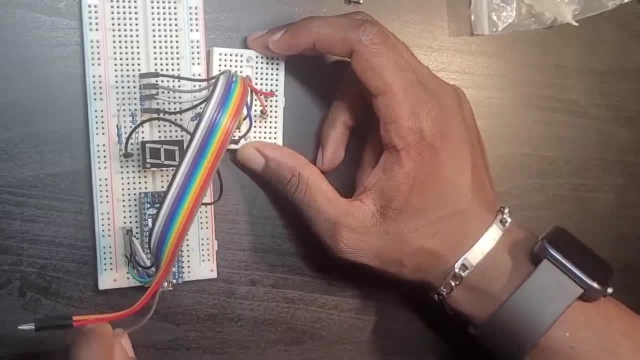 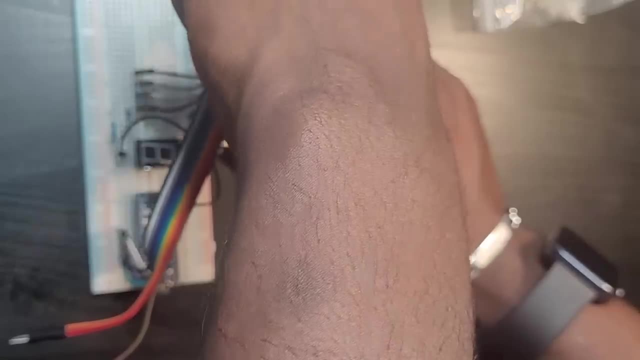 See what I did wrong here. Instead of connecting an orange pin, I connected a brown pin. here. The brown is the very, very edge. I'm not supposed to do that again, So I made a mistake here. Let me just solve that. 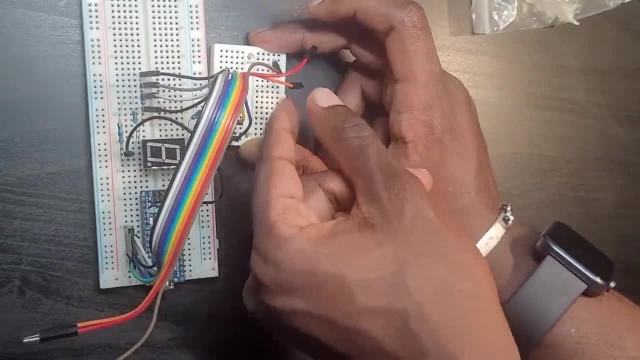 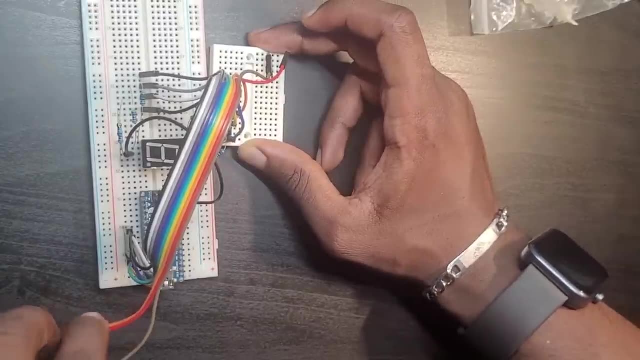 Remove the brown And what is next to yellow? It's orange. I'm supposed to be connecting orange. I made a mistake, My bad, And there we go. Now I fix it And now I also connect the orange from this side. 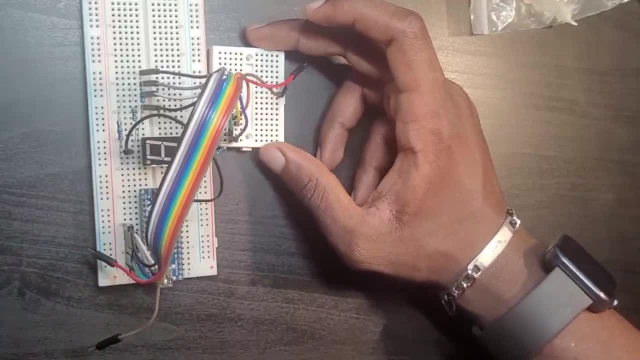 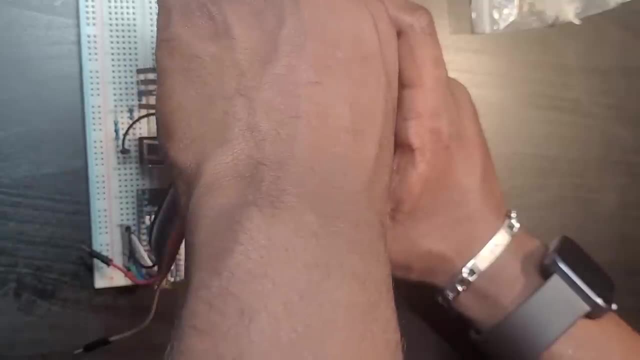 Okay, Now everything seems to go. Okay, Everything seems to be right. All right, let me just again connect these two pins so that they hold the small breadboard together. I'm just going to kind of put it here so that it does not move a lot. 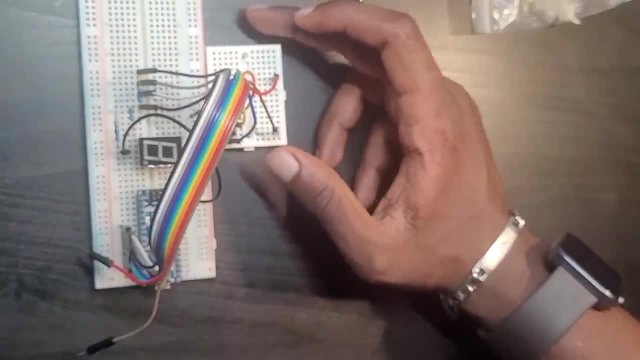 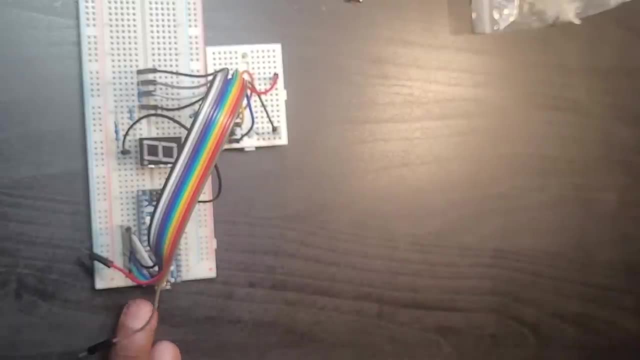 Again, they have no purpose other than holding the breadboard, the red and the brown pin. Okay, So now I think the wiring is right, And now I set up what? Everything. the name is right. It extends to what To 10, from two to 10.. 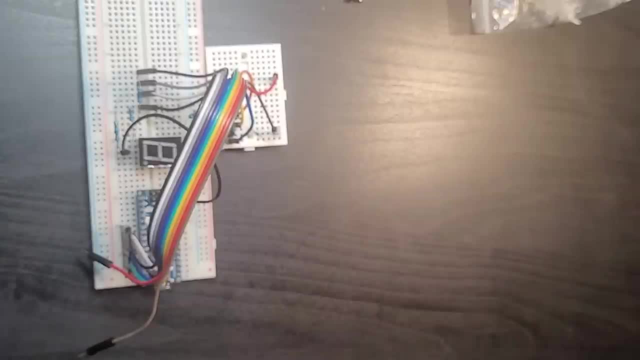 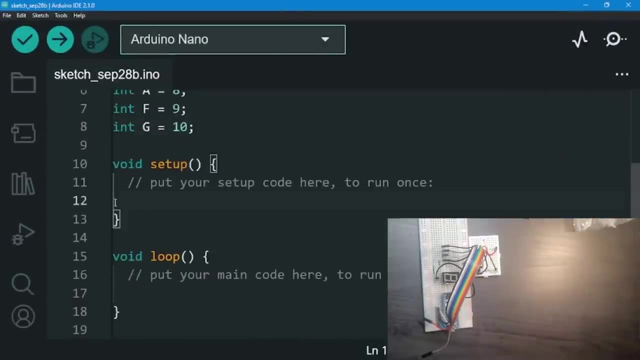 So everything seems to be correct. from so I said two, I meant three, three to 10.. So everything seems to be right. So now let me go over to my code. and now let me just go to pin mode and set everything up. pin mode: set everything up. 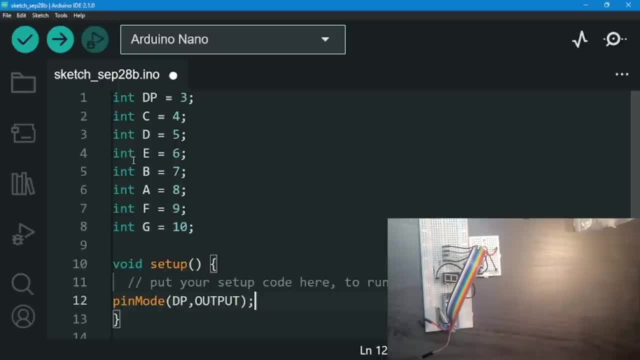 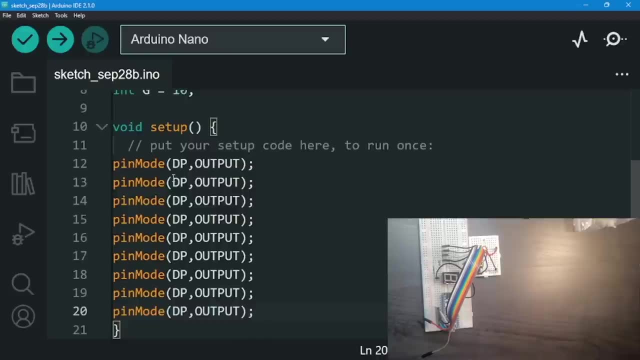 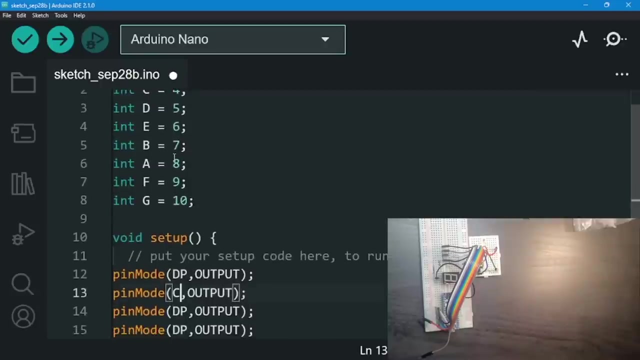 So we have decimal point. set it to what? Set it to output. All right, Keep copying this. alternate shift down. keep copying it and then I can do what I can change the names. So I'm going to start with CDE. 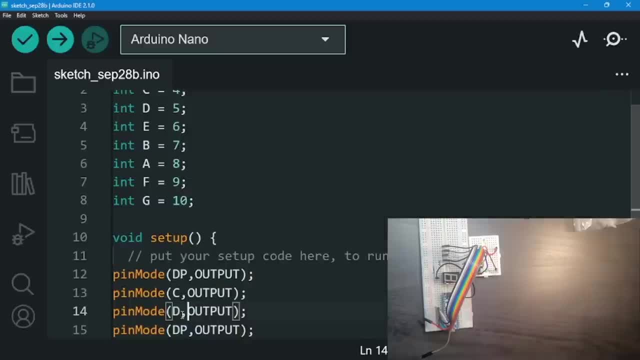 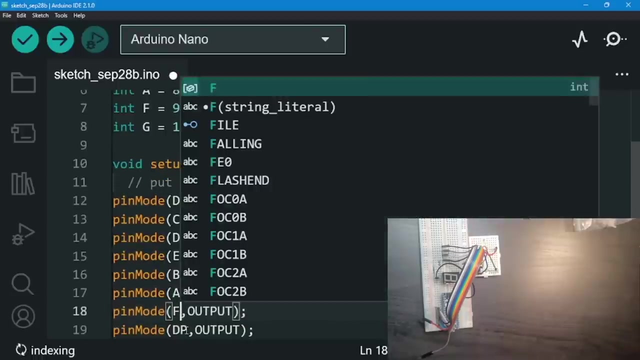 Let me just go C, And then there's D, And then there's what, There's E, And then there's B. Let's go to B, And then there's what? And then there's A, And then there's F, And then there's G. Okay, 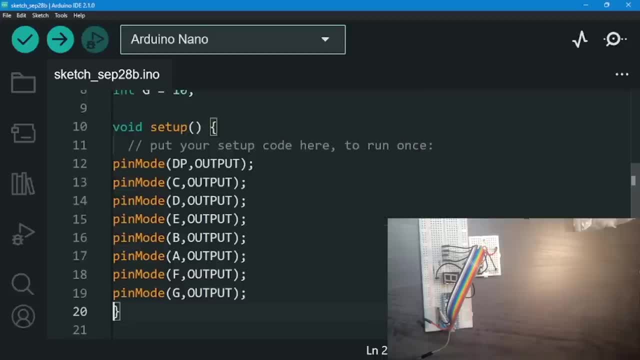 Let me just remove the final one. Let me just count the pins. They're supposed to be eight, One, two. let me just count it: One, two, three, Four, five, six, seven, eight. There are eight pins. 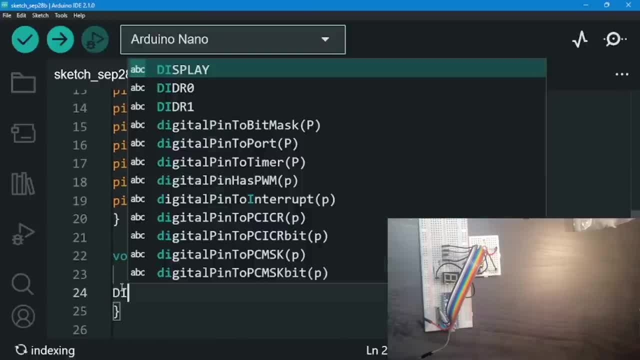 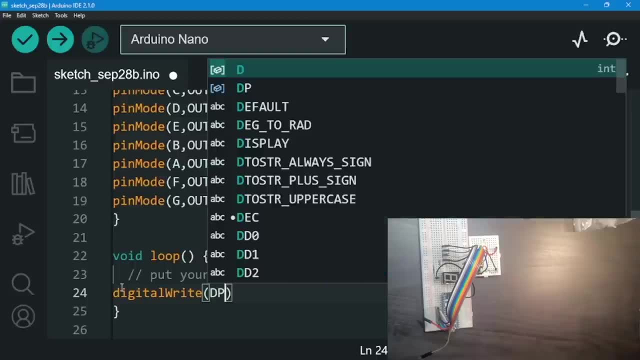 Okay, Good, Now what do I need to do to light up? everything I'm going to need to do is what? Use digital, write Okay And set my pin right here. Let me just start again. Decimal pin And set it to high. 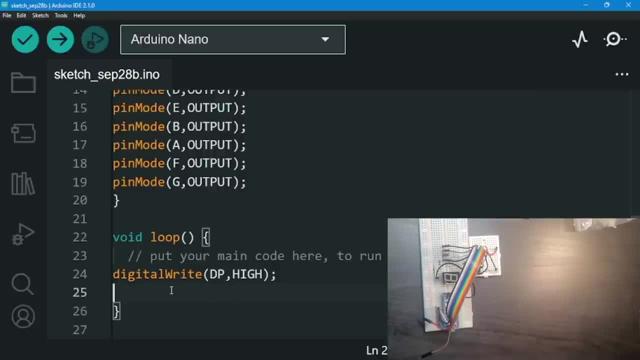 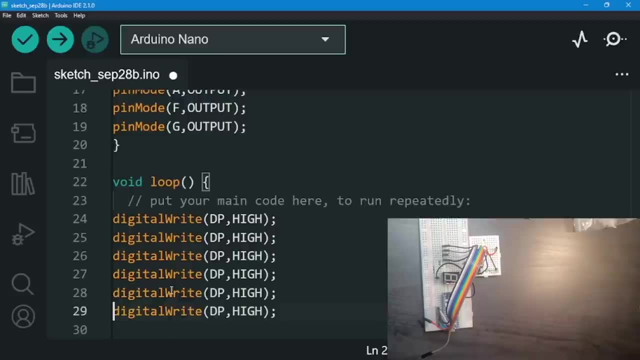 Once I'm done with that, to light every component. right now, what do I need to do? Again, I'm going to need to write the digital write And we need to copy it. It's going to be second, Two, Three. 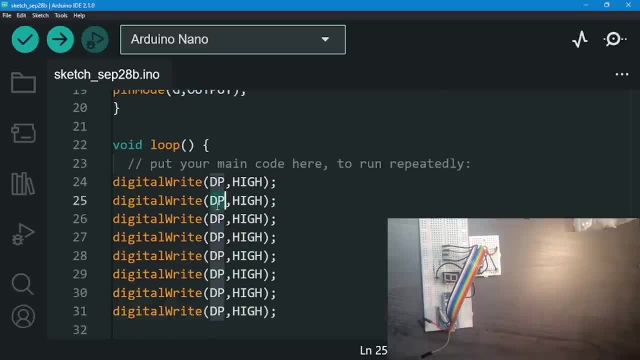 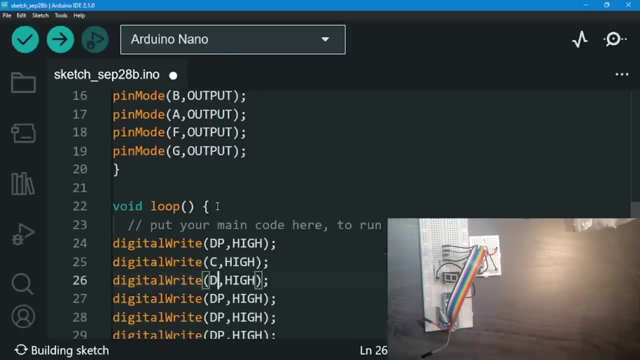 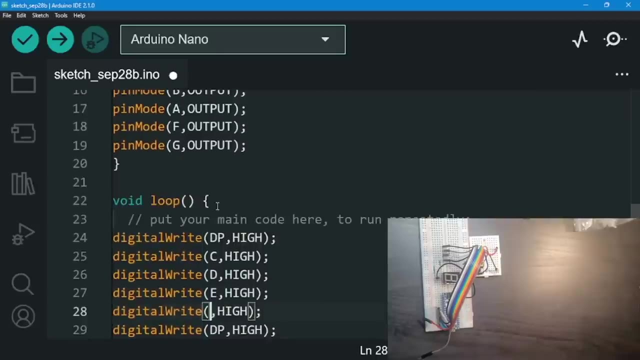 Four, Five, Six, Seven, Eight. Okay, Now, where do I go? Now let me write them down: C, D, E, C, D, E, And then, after E, there's B, A, B, A. 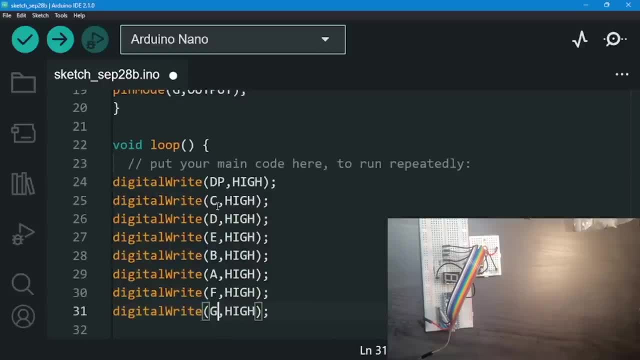 F, And then finally G. There we go, So now, let's just upload it. I need to upload it, though. What do I need to do? I need to wire up my Arduino, So I'm going to move this again slowly. 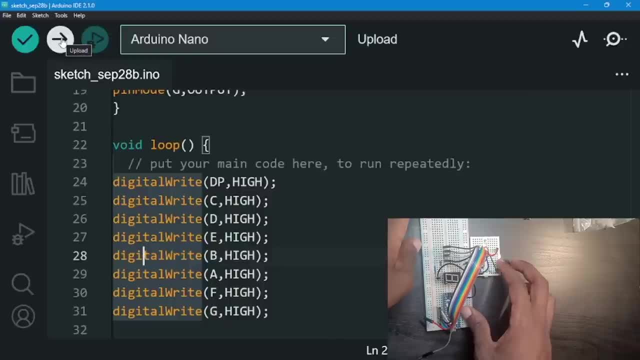 It's going to be a bit of a hustle because if things go wrong right now and the resistors go wrong, it's going to be really, really sad because the amount of what wiring it took, I'm going to attach both and slowly move it again. 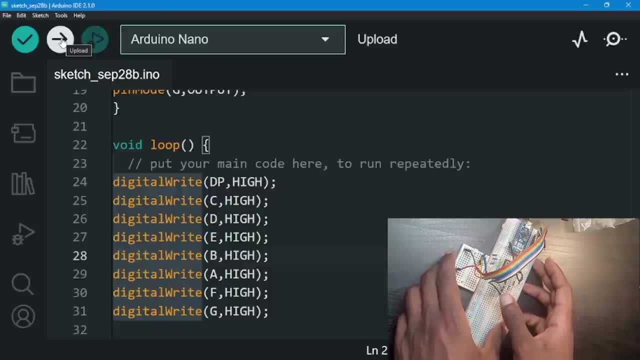 Need to be gentle, Very, very gentle, Because these resistors again can just pop out. really, Just push it a bit. Okay Now let's just try to turn on our Arduino. Okay Now, let's just verify our sketch. 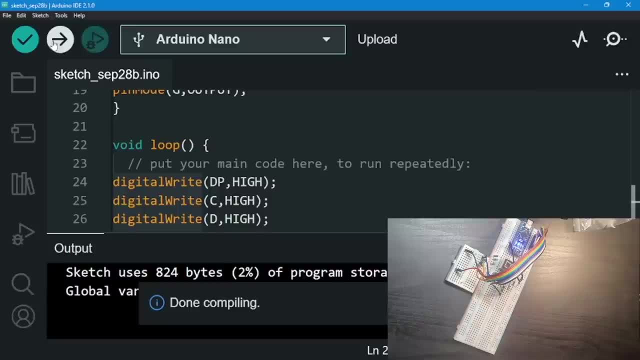 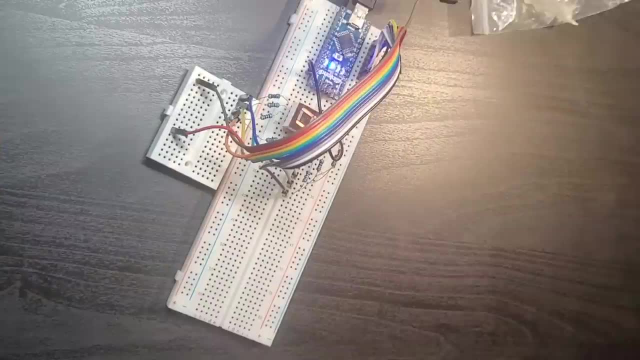 Let's do that: Verify my sketch. Hopefully everything's good. Okay, That's good. Now what? Now I can just compile it. It's compiling And now it's done uploading. Okay, Can you see it? It's not fully lit enough. 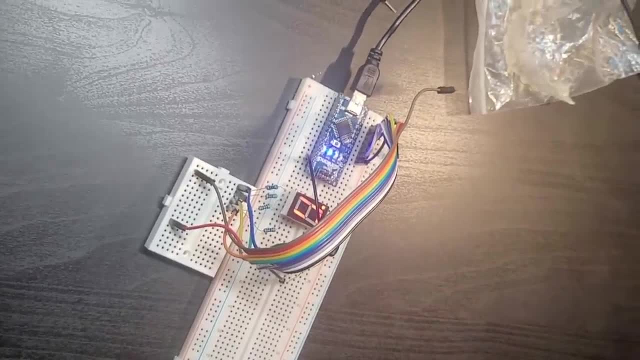 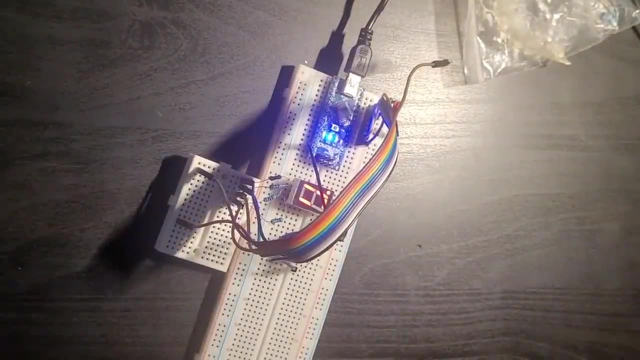 I just need to move this a bit. Okay, I'm just going to move it a bit so you can see it. The wires, There you go, Let me just focus on them. Let me just turn off the one light right here so you can focus at it. 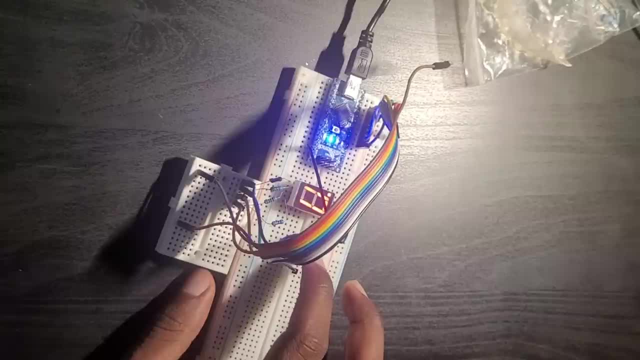 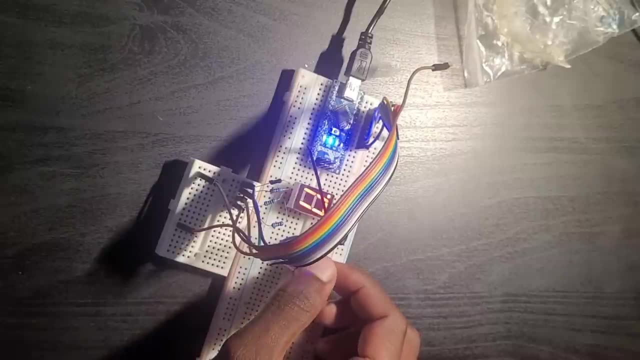 Not everything is turned on. Why is that so? Just the resistors again. Let me just: if I touch one resistor right here, look at it. If I just touch one resistor lights up, It's because the resistors are not connected properly. 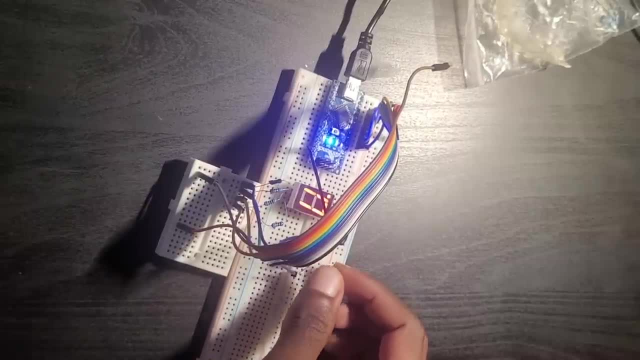 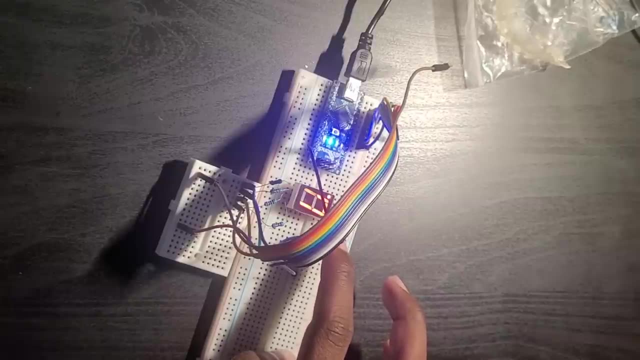 Okay. So let me just again Push the resistors a bit. There we go: Push this one in. This one is pushed in properly. Everything seems to be intact here, All right, Okay, Let me just check the other resistors right now. 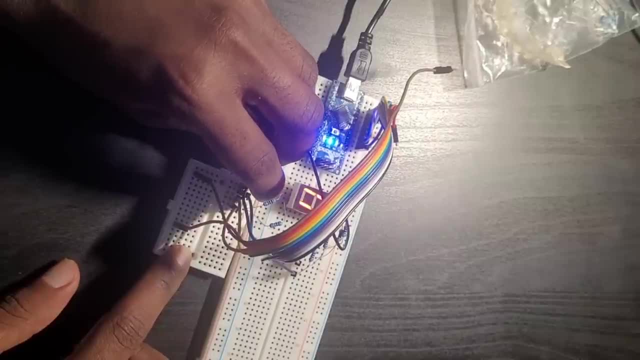 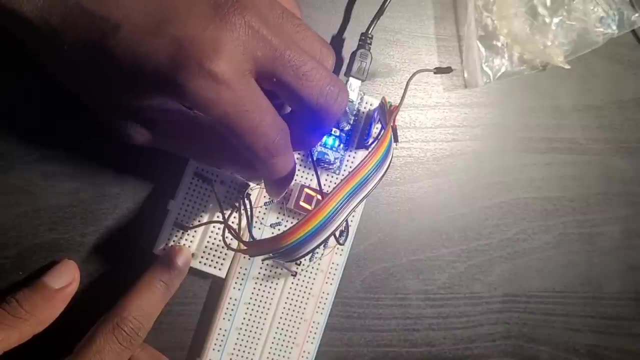 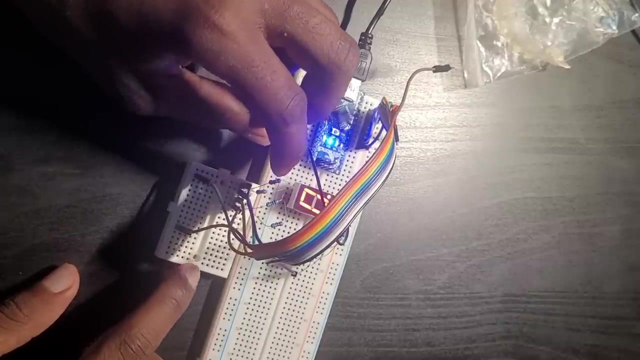 Oh, there we go. Can you see it? The second resistor is not connected properly. Slowly, We need to go slow. It's moving a bit too fast. Just push it. Just push it. Okay, There we go. How about this one? 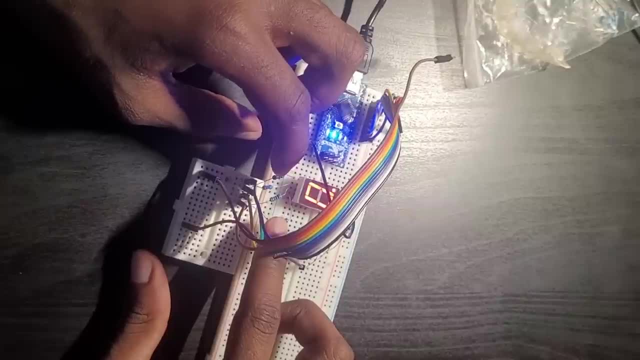 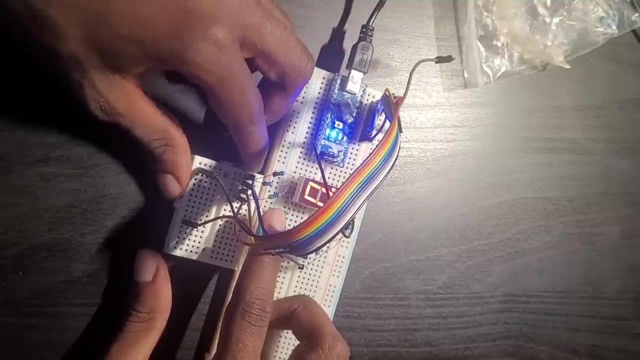 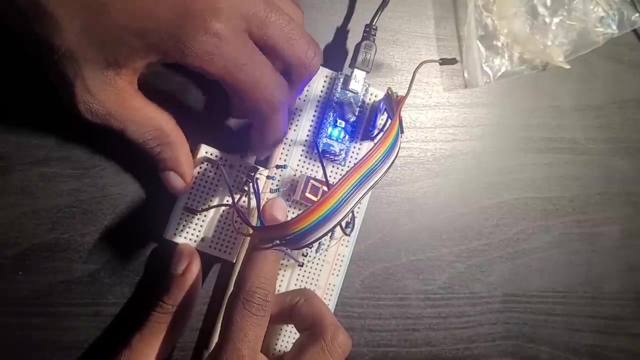 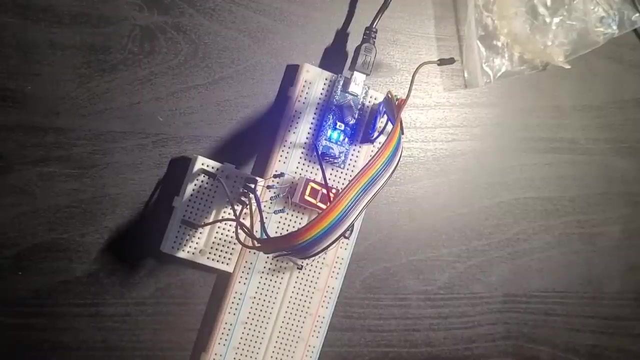 The G pin, I think is the very left one, because I put it at the very edge, It's not lighting up. Okay, this PID, There we go. Let's push this. It's a bit of a hustle. Let me try to push in this. 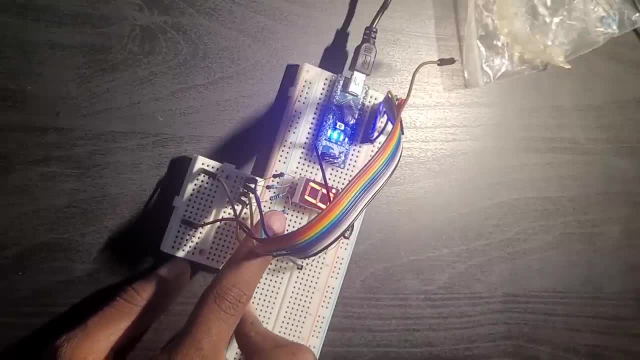 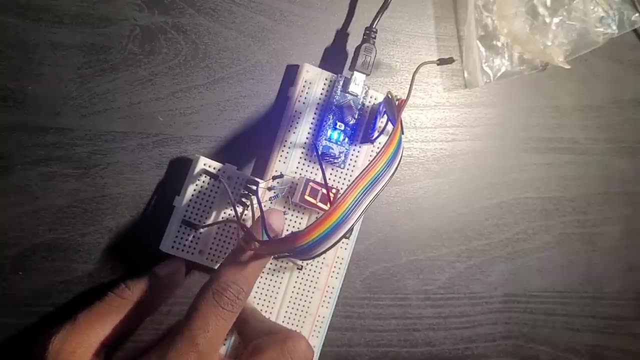 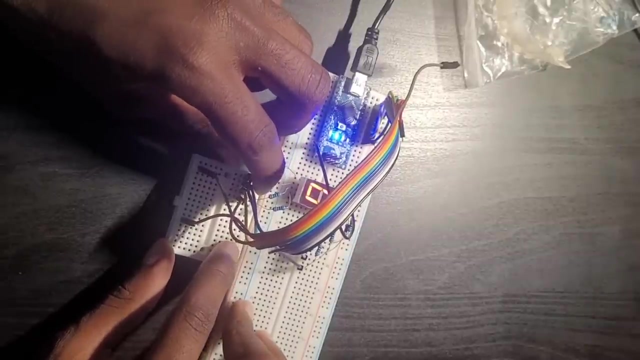 one. And what is not lighting up? What segment is not lighting up right now? Okay, this segment is because of this resistor. This resistor seems to be working, fine. How about this resistor? Okay, both of them, okay, I see. So again, wiring it up is a big problem in itself, especially. 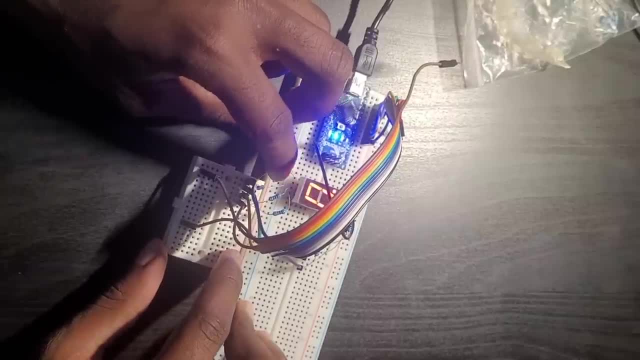 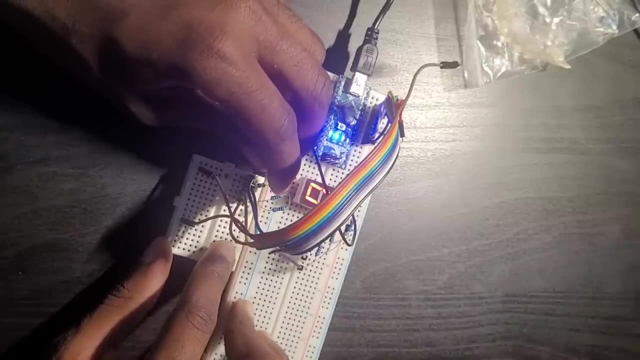 with these resistors. They don't hold in place, and I find it really hard. Can you see that? Okay, so they're not holding in place. So what I'm going to do is again fix the resistors. This resistor- let me just see if this is even correct, because not all of them are. 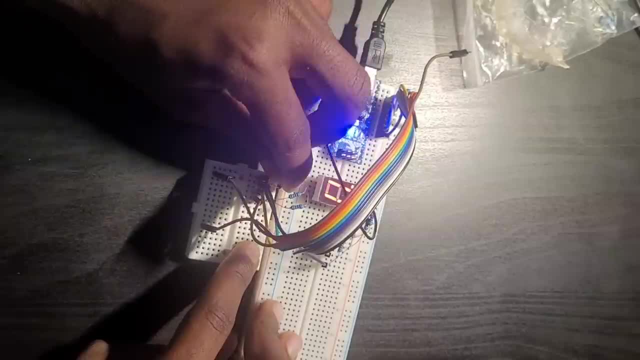 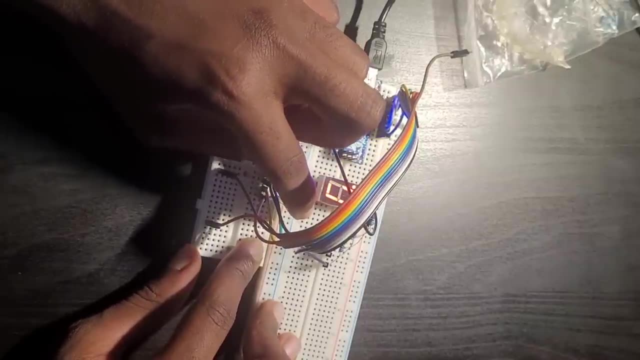 on Just again, so you can see that not all of them are on. So let's see if this is even correct. Not all of them are on. So for those of you who are using a digital Arduino, it's going to be really easy. for you guys, It's going to be way easier than here Again due. 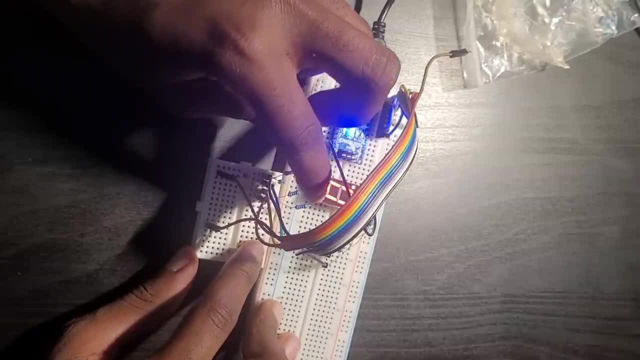 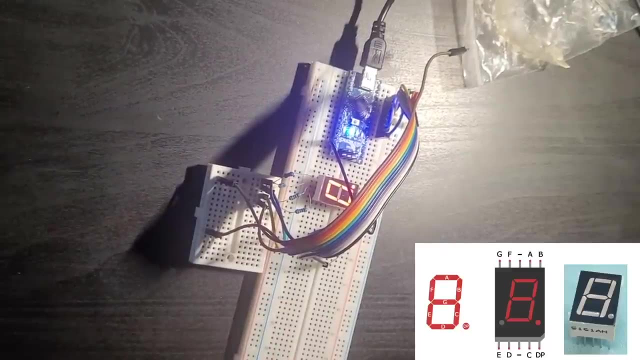 to the limitation we have again in components, we're going to have to find a way to work around it. Okay, everything seems to be working fine, but the middle pin right here. Let me just check what is even the name of the PID. Let's just check the name of the PID. Okay, 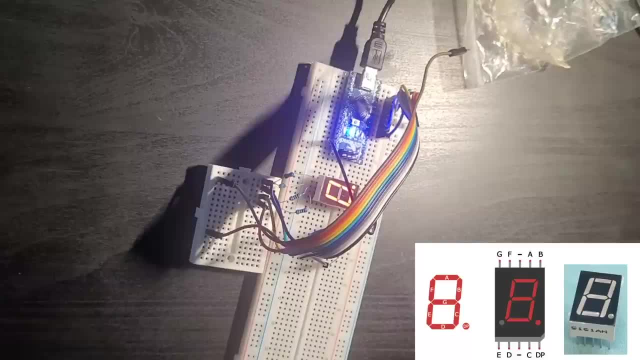 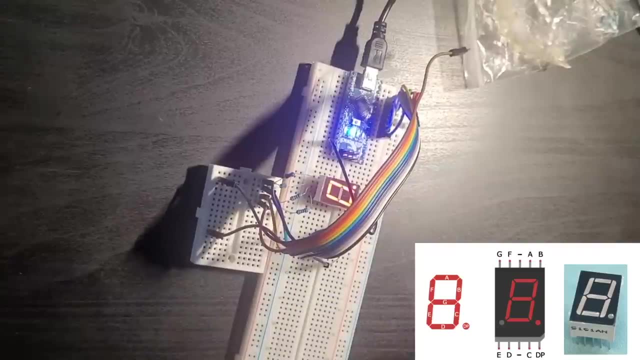 so let me go to my Chrome. The middle pin is the G-PID. Where is the G-PID? Which one is connected to the middle pin? How am I supposed to know that? Let me again check the image. G is supposed to be around here. Okay, G is around here. G is at. 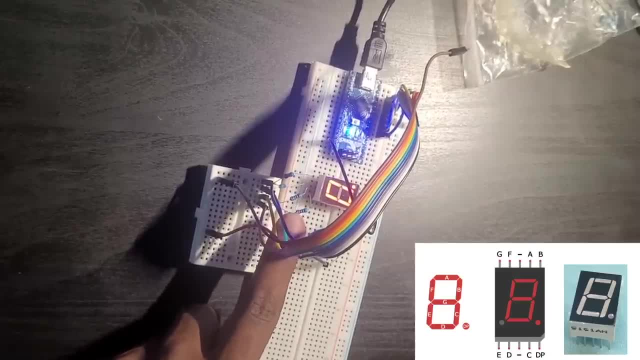 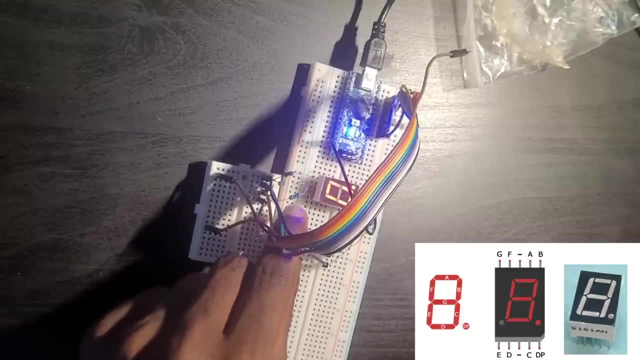 the very edge, The very edge, but the resistor at the very edge is not working. basically, Let me just check. even if it's wired up correctly, I just need to remove this. It's not doing much of a thing Slowly. 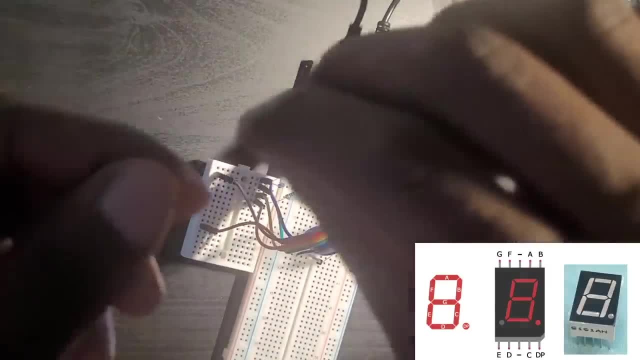 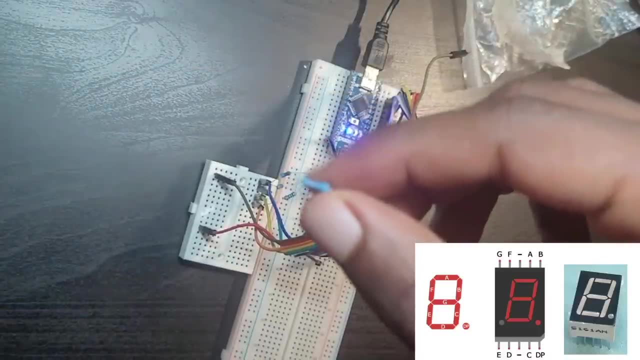 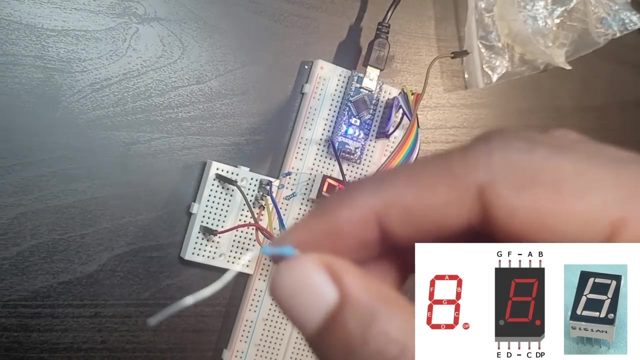 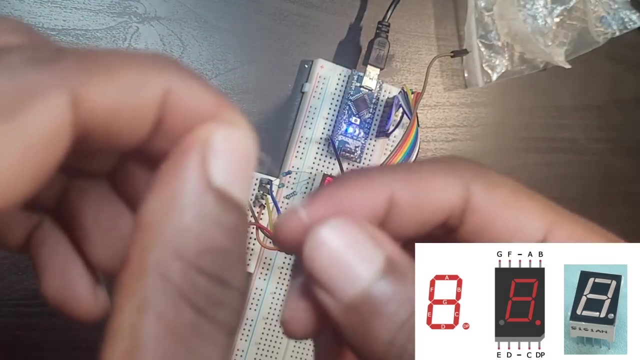 Okay, let me just again straighten out the resistor. Hopefully you can see it. I'll just bring the light off. Let's make a focus on the resistor. The focus is bad. I'm just going to straighten out my resistor. I'm just focused on the LED right now. Okay, straighten it out. 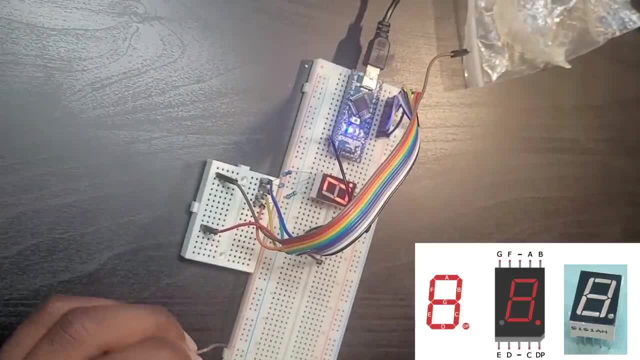 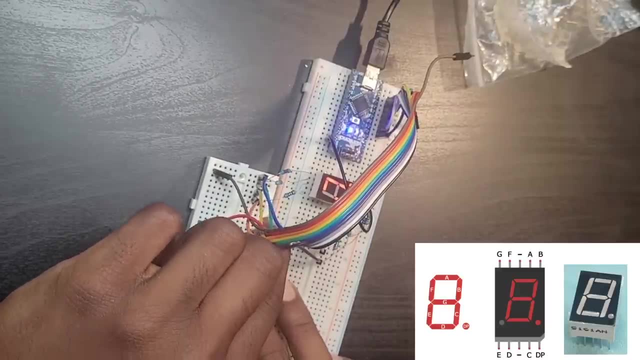 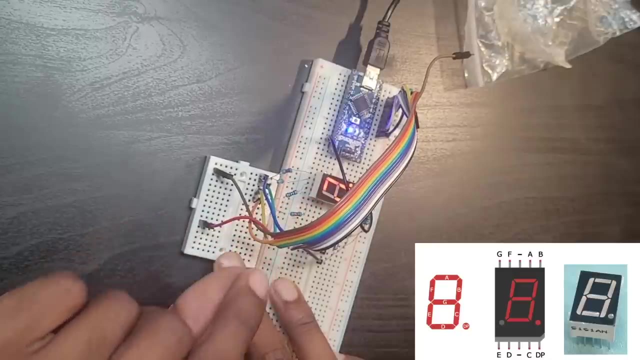 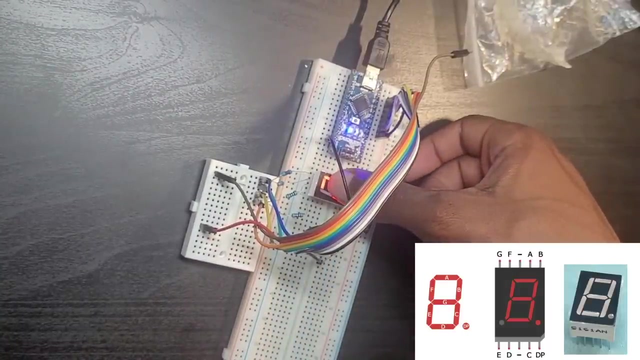 There we go. Now I'm going to have to carefully put it back in Just again. hustle, Let's do that. Oh, I see the problem here too. I did not push it in. Let me just push in my LED. Just push it in. 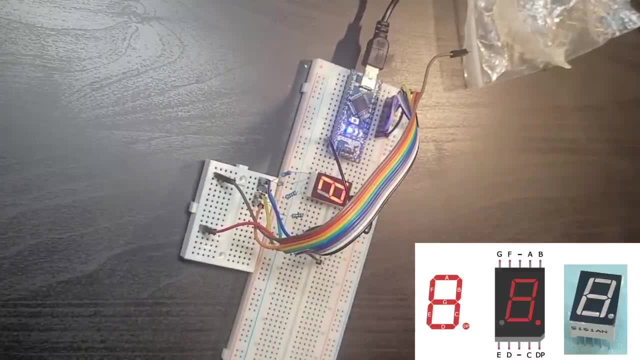 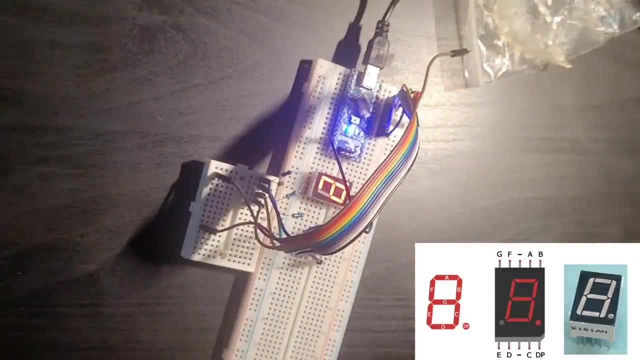 first. There we go. Now it's pushed in, Our LED is pushed in. Only what? Only one line is not. Only one line is missed. right here I can turn off my light so you can see it better. Only one line is not, It's not. 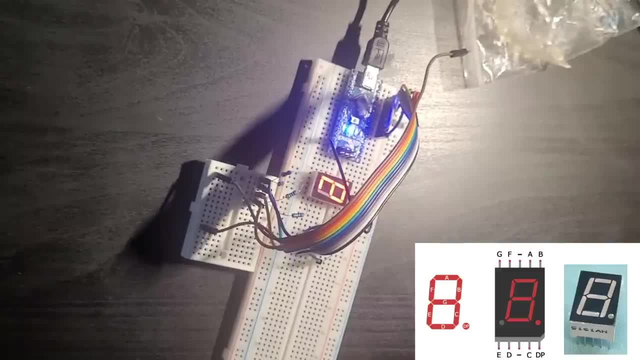 appearing. What is it? It's the line F. It's going to be next to what? Next to G. So the resistor next to G is not lighting up properly. Let me just check why it's not lighting up properly. I'm just 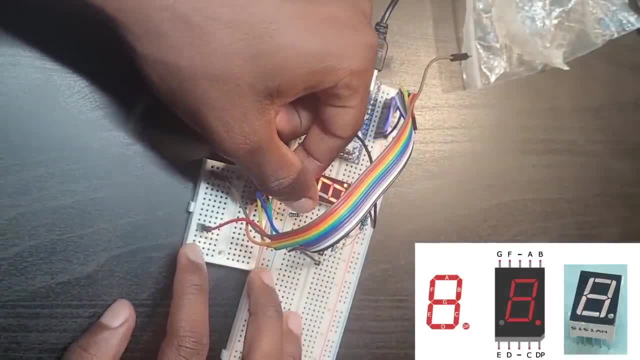 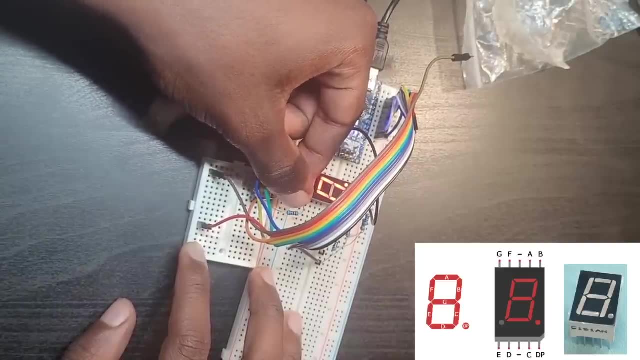 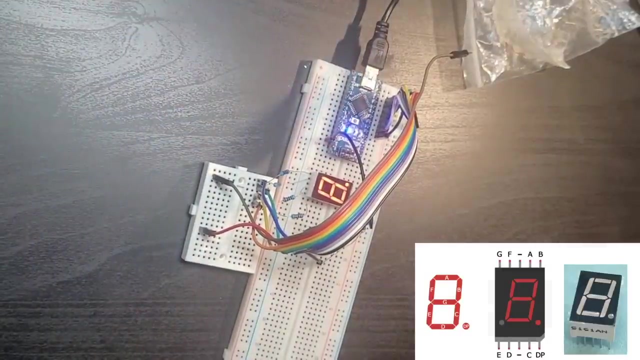 going to turn on my light right here. It's a bit of a hustle, as I said again. Oh, I see What the problem is There. we go Push it in and then slowly let go, Slowly let go. Let me just. 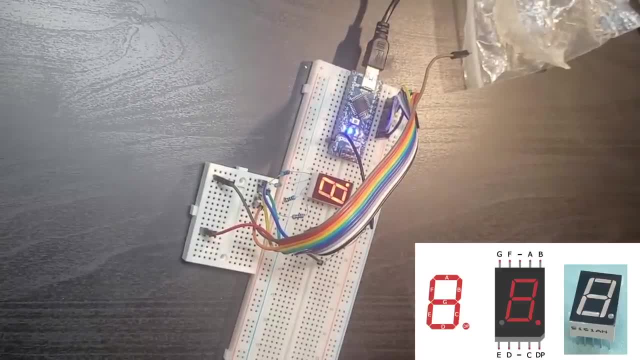 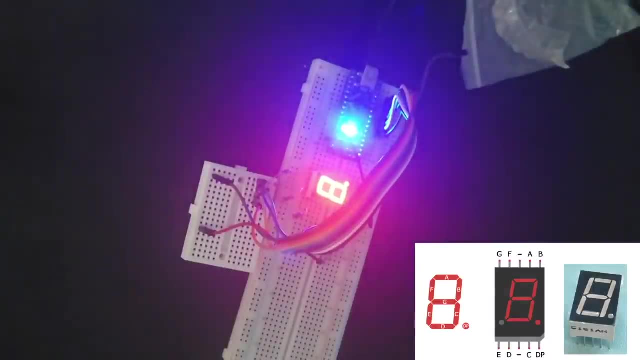 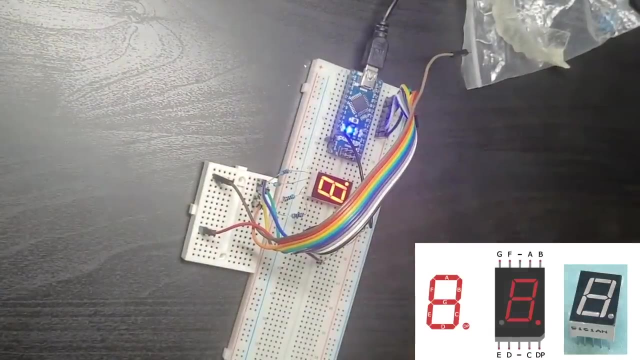 turn off bulb light so we can see what we did right here. It looks beautiful. Okay, Turn it off and turn it off. Let me just turn off the other one. There we go. Now everything is lighting up, including the what The decimal point. All right, Nice, Okay. 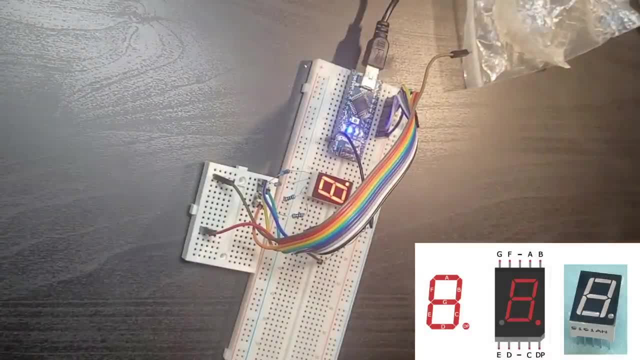 Let me just go right here and do exactly what I just did. I'm going to light up two or three pins on the common anode. I'm using a common cathode, so I'm going to show you guys how to do it in a 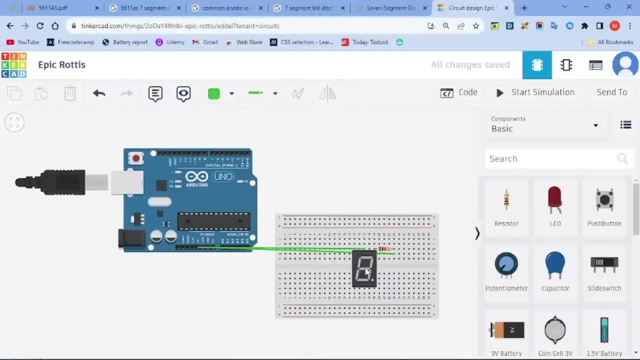 common anode, just in case you do not know. Okay, So let me just go right here. This is a common anode, as I said, So let me just turn this off, Let me just take this off, Let me delete this. 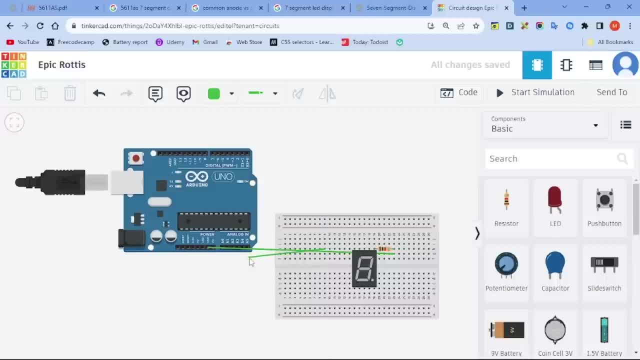 first, Where's the delete button. There we go. Let me just first read it. There we go. Okay, Delete this, Delete the resistor. So basically, what do you do is what We have a common, what We have a common anode. So what do we do? We have a common, what We have a common. 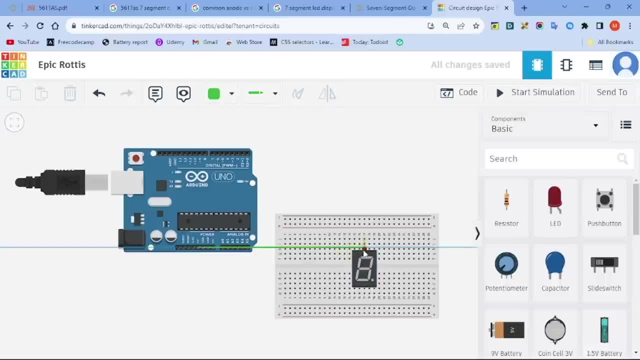 5-volt. So what I'm going to do right here is connect the 5-volt right here, the common 5-volt, to the third pin. Again, I can use the one that is at the bottom right here or I can use the one. 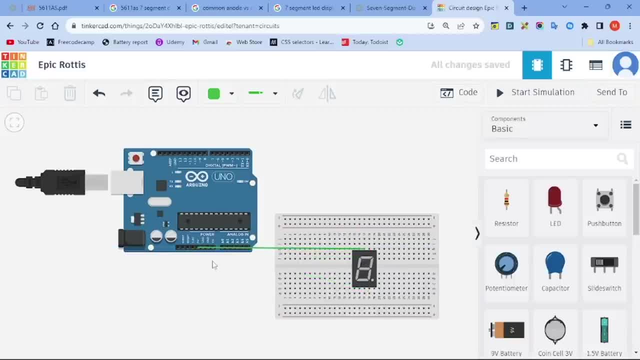 at the top. It's up to me. There we go. Now, once I'm done connecting the 5-volt, I'm just going to give it a color right here so that it's easier to see. So let me just turn this off, Let me just 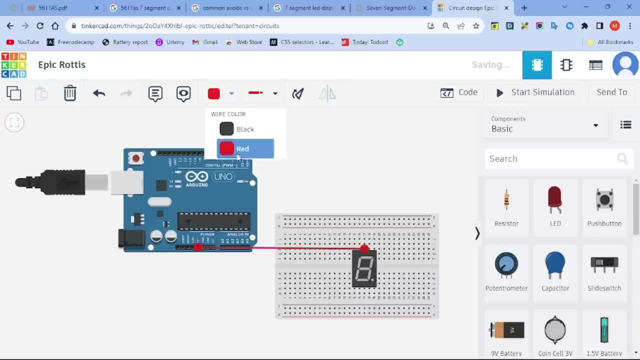 change the color right here to red. There we go, The 5-volt, And now I'm going to start connecting what I'm going to start connecting using resistors. So let me just connect one, Let me just light up. 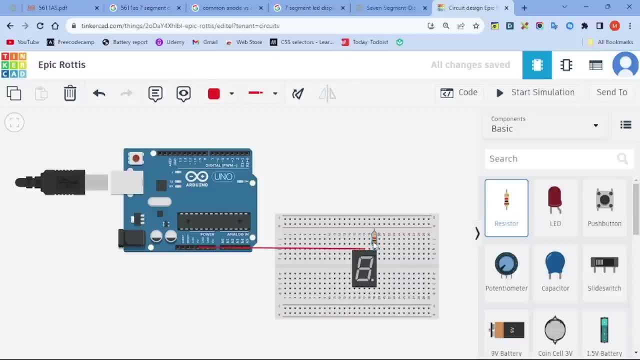 one, two, three segments, And then I'm sure that you can do the rest of it. Okay, I'm sure that you can light up the rest of it, So I'm just going to go right here. It has a resistance of 1 kilo. 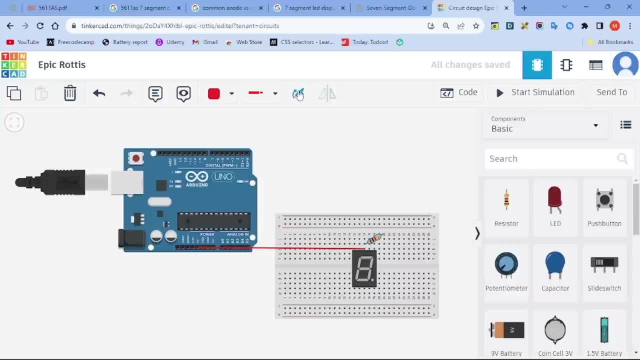 ohms. Okay, Basically about 1,000 ohms, And now let me just rotate it. Just rotate it right now. Okay, So you might be wondering how to turn it on using a digital pin. All we did was what? Just a. 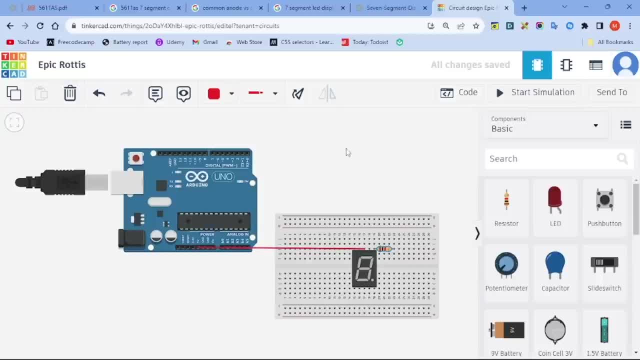 5-volt and the ground pin. So I'm just going to show you guys how to use a digital pin and just light it up. Okay, We can get another resistor here. Let me just light up this part too. Okay, Just rotate it Right. There we go. Let me start writing code for this. So. 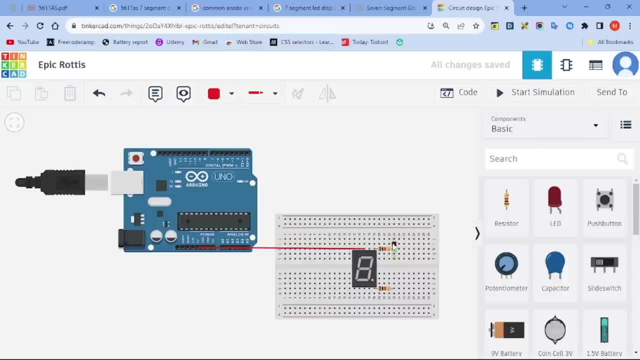 before doing that, actually I need to connect the wires. So I'm going to connect this wire right here to digital pin 3.. Let me start from pin 3.. Just give this another color. Let me start with the orange. There we go, And let's give this another color too. First, connect this to digital. 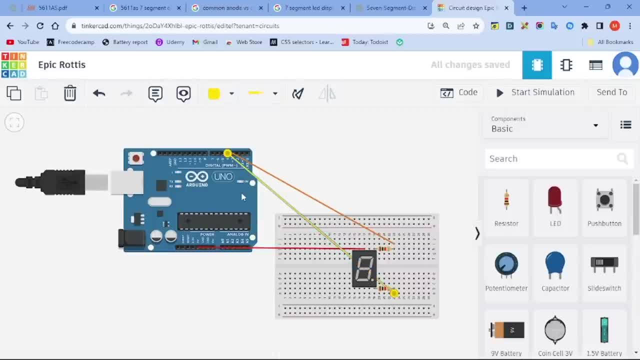 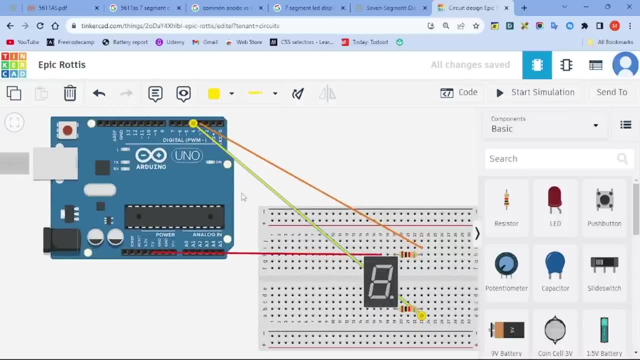 pin 4.. There we go, Give it another color so you can see it way better. I'm just going to zoom in so you can see the circuit way better. Okay, There you go. That's the circuit that I'm going to be. 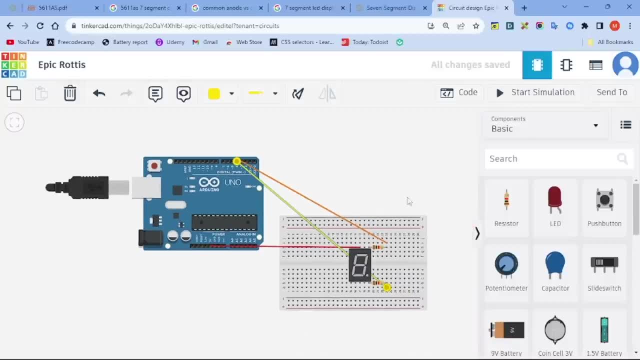 using. You can pause the video and check it out, So I'm just going to zoom in so you can see the circuit. Take it for yourself. Okay, All right Now let me just go to the code. So what you need. 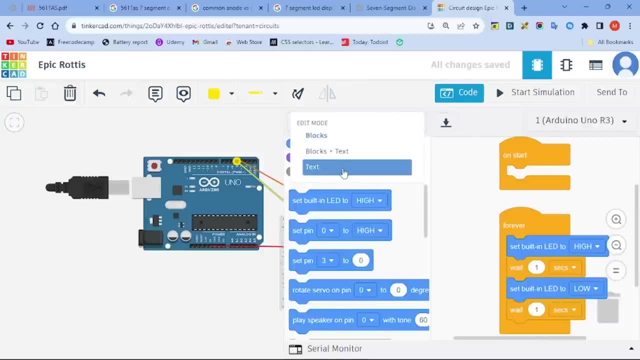 to do is basically the opposite. when it comes to what? When it comes to the common what, The common cathode, Okay, So I'm going to go to text, I'm going to use text. So what I'm going to do is: 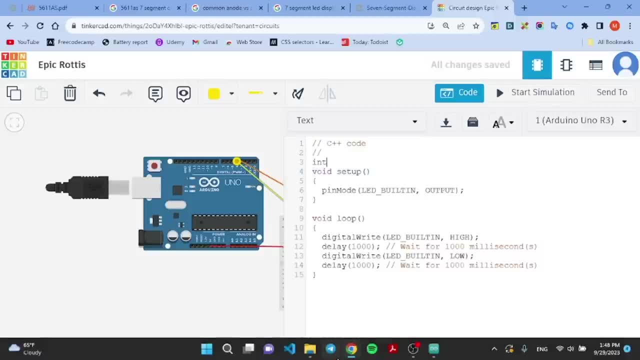 let me just again set up variables. I want you to do it yourself For those who have common anode. I'm sure you guys can do it. You just have to follow the same step, but there's going to be a difference. I'm just going to show you the difference here. Okay, That's basically what. 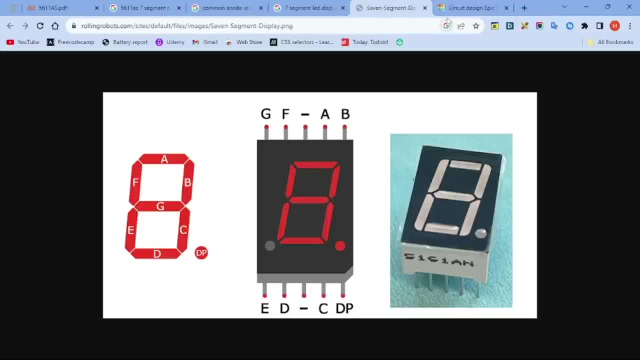 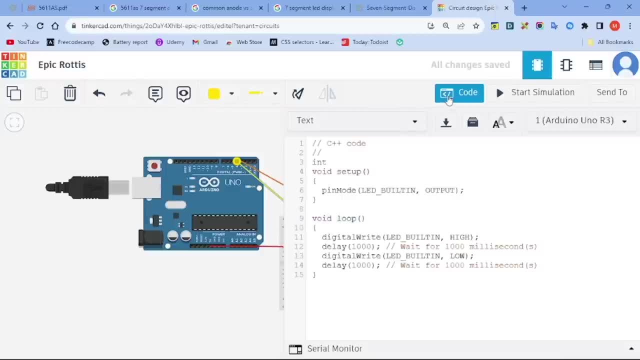 you need to do. Let me just bring the seventh segment. Where is it, The seventh segment image? I'm going to be connecting B right here. Just see it, It's going to be. let me just take off the code for now. I'm going to be connecting B. 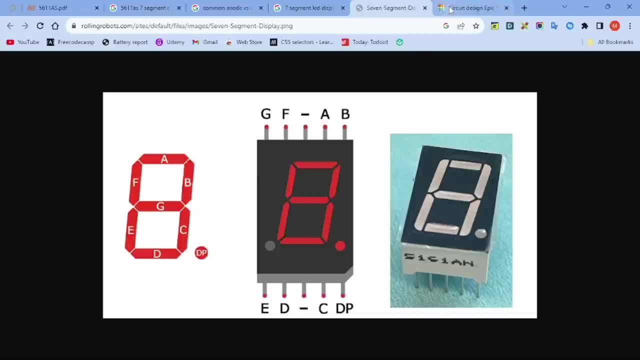 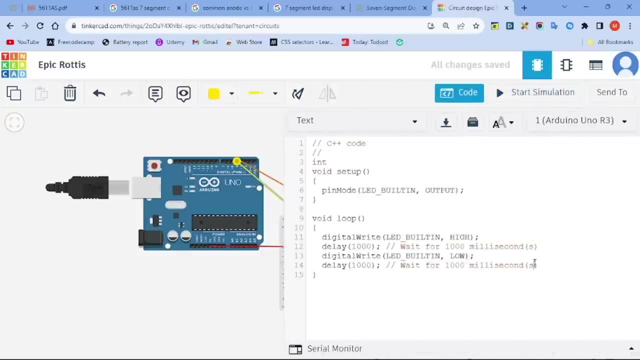 and from underneath. here I'm going to be connecting what. I'm going to be connecting the decimal point. Okay, I'm going to connect the decimal point and B. Where is B? B is around here. I'm going to be lighting this and this up. Okay, So let me go to our code. Then what? Let me just 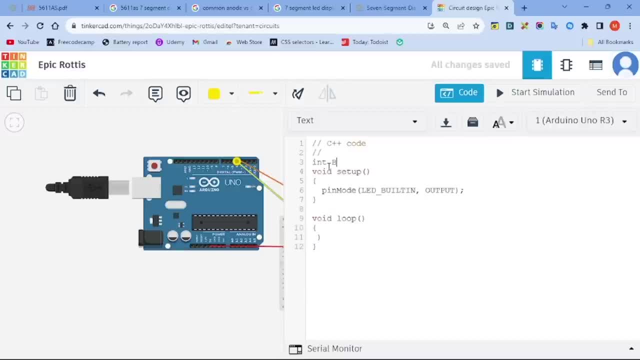 pull this code right here. I don't want that. So I'm going to say B- What pin is it? It's pin 3.. It's going to be the digital pin 3.. And what do we have? Decimal point. It's going to be connected. 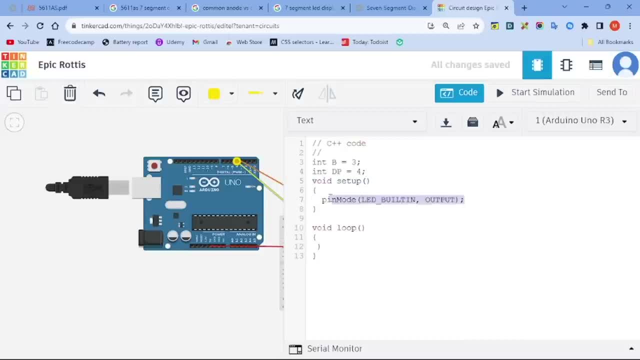 to what To what, The digital pin 4.. And what I need you to do is what? Right here, set it up as we did normally. I've set it up Pin mode. set B to what The output, Just get the capitalization. 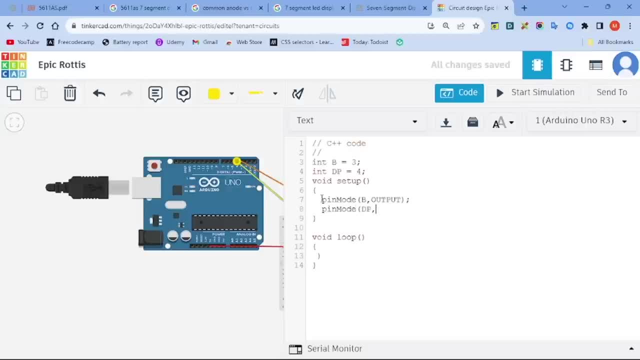 right Pin mode. set the decimal point 2 to what To output Output. There we go, And all you need to do right here is, instead of using digital right, again, we're going to be using digital right and setting it to high. What you're going to be setting it to is low. Okay, We're going to be. 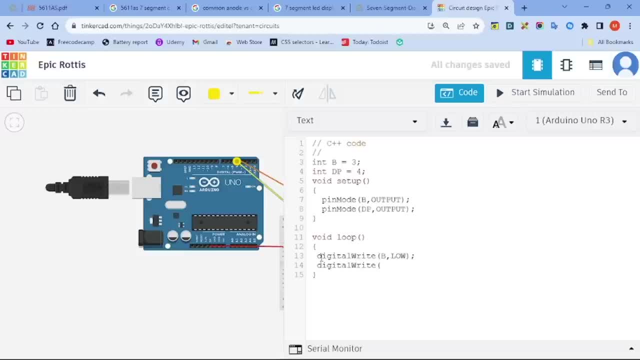 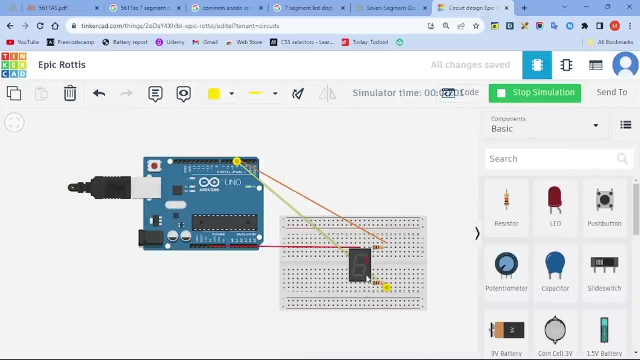 setting it to what? To low, Basically, almost acting like a. what It's going to act like a GND pin. Okay, So I'm going to do decimal point and setting it to low. So let me just start the simulation right here And let's move our code And there you go, B and 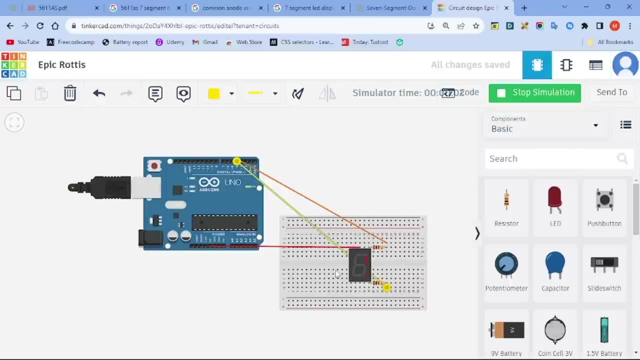 decimal point is what They're activated. So what I want you to do, again to light up everything is what? Again, connect all these components yourself, Just like how I did using my common cathode. Again, connect it And then write every code, Obviously for common anode. you're going to be. 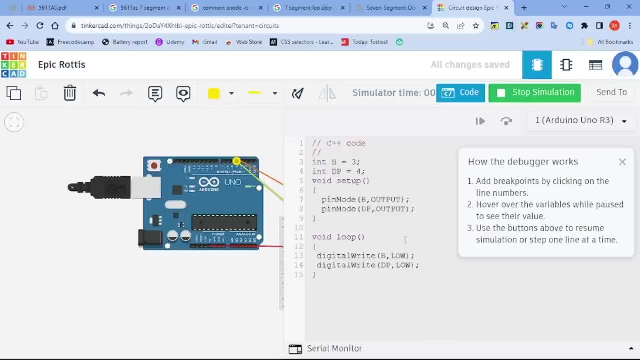 using what. You're going to be setting it to low, Okay, That's all you need to do. Instead of high, you're going to be setting it to what? To low, Okay. So now what I did is what. What I did is set it up to what To light up everything, So to even. 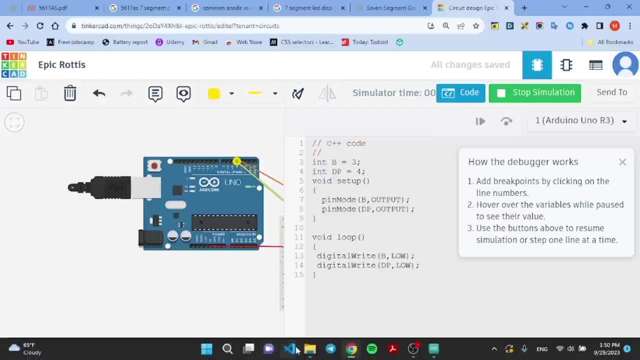 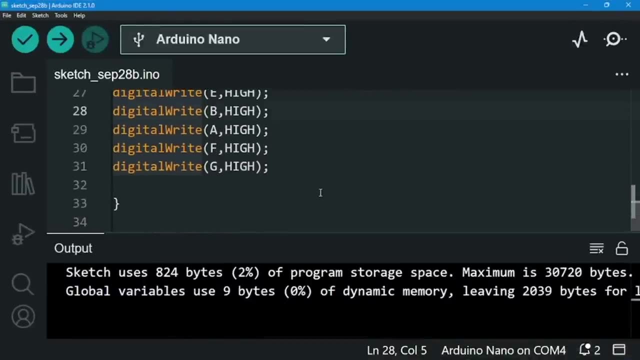 make a timer. right now, let me go over to my Arduino IDE. There we go. So now, what do I need to do? I want to set it to what I want it to count from nine, then go to eight, then go to seven. 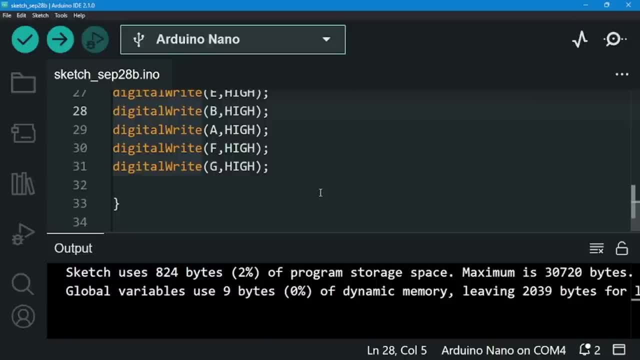 six, five, four, three, two, one, and then finally going to what? To zero. Okay, That's what I wanted to do. So again, I turned all of this just to check that everything is connected. I turned off everything to high just to see that they're connected. And now they're. 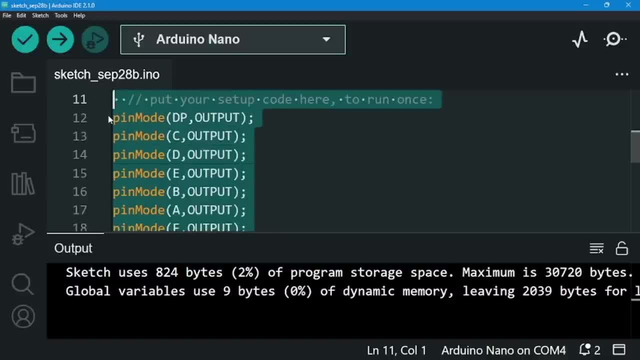 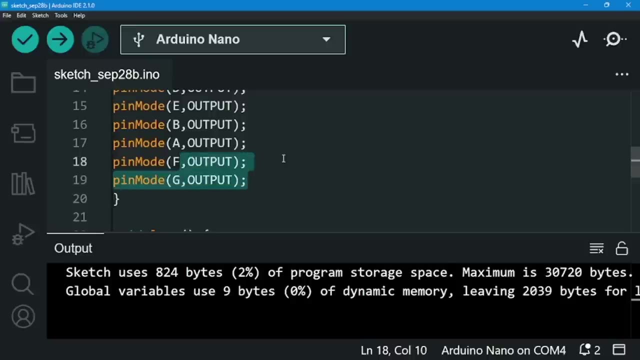 successfully connected because everything's on. I just wanted to check if everything is on so that it does not give me, does not cause me problems later on. Okay, Oh, I just turned off the pin mode. Sorry, I was supposed to delete the high ones. I accidentally cut this. Sorry, I just put. 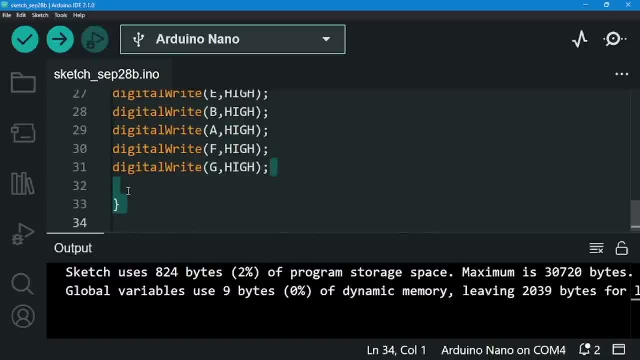 my pen to high, but I didn't. So now, what do I want to do? What do I want to do is what? Take off the digital lights, not the pin mode. Pin what I did. It's a bit of a hard drive. There we go. 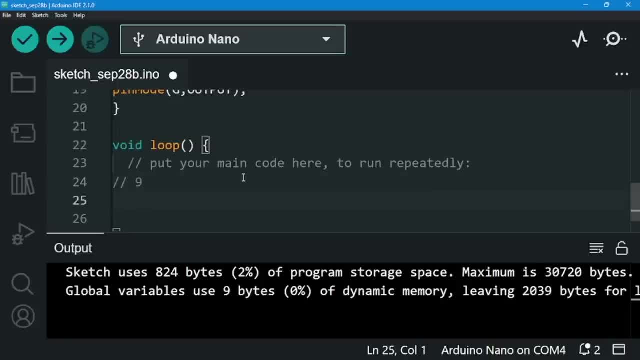 There we go Now for nine. what do we need to light up for nine? We need to light up what? So let me start from here. I just copied this. okay, What I want you to do is what? Before cutting this, 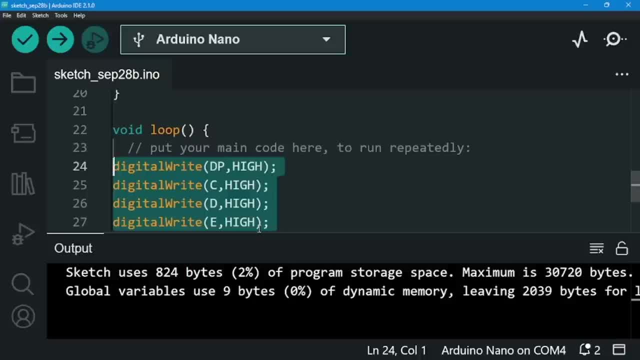 okay, I want you to copy it again, that I set it to all of it, to high. I want you to copy it, that you want to just turn this off, and then I want you to copy this, Okay. So what I want you to do is: 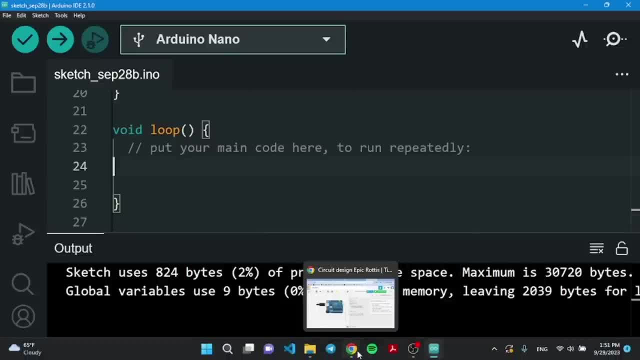 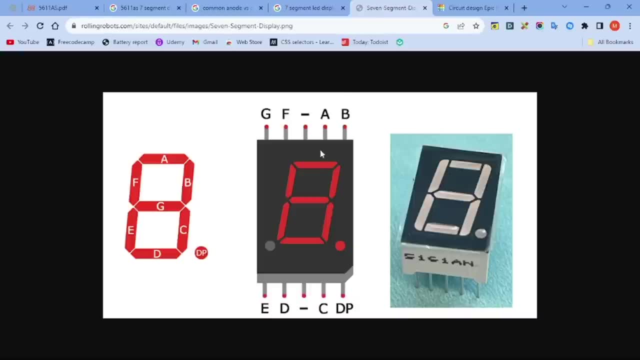 turn it off right here. what i want you to do is for nine. what segments do we want to light up? so we go over right here. you want to light up what we want to light up. where is nine there? we go for nine. we're gonna need to light up what a, b, g, c and d- a, b, g, c and d. so what i'm going to do? right. 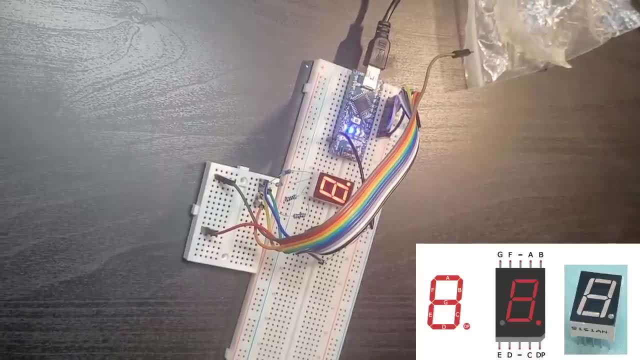 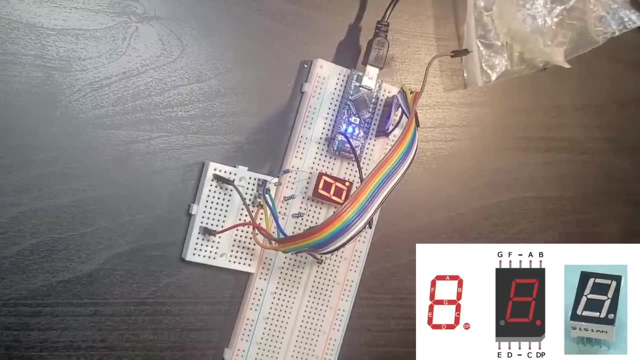 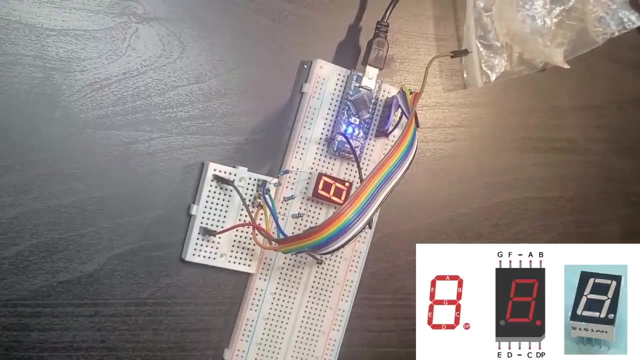 here is: bring a paper. i think it's going to make it way easier. let's first write it down. i think it's better that way. so i'm just bringing a paper right here. i need some paper. just go get it there. we go. all right, there we go. found the paper right here. let me go get my sharpie. 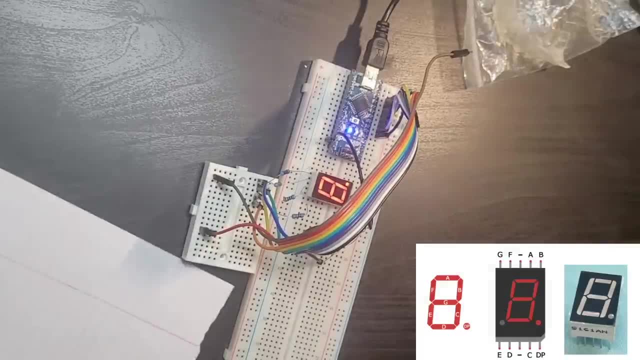 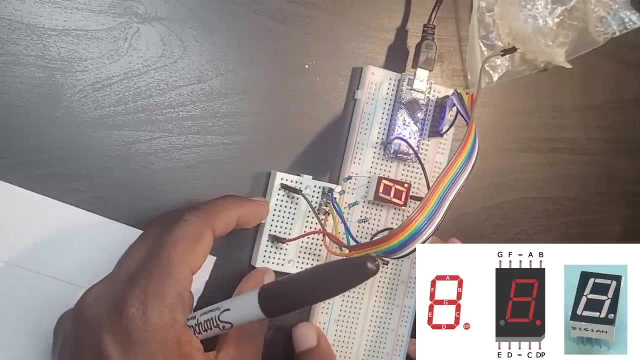 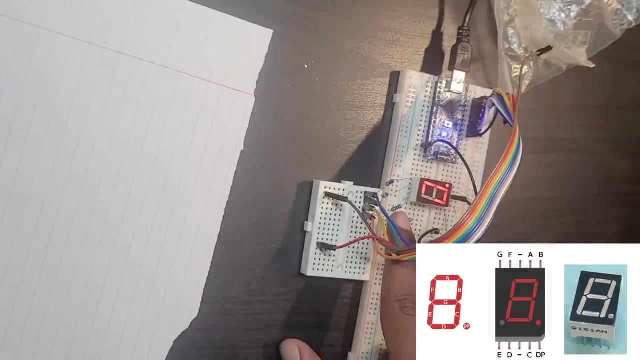 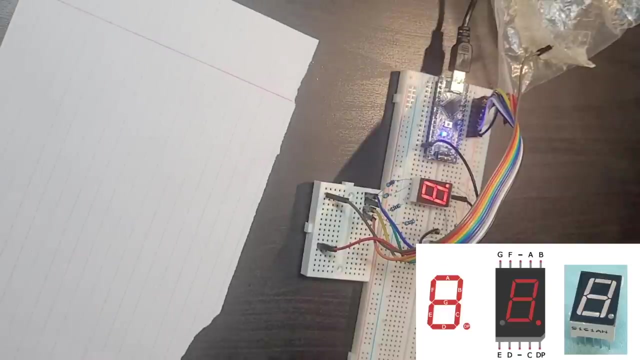 where's the sharpie? there you go, found my sharpie. i don't want to push this a lot, so just slowly move it because i need that space. oh my god, it's very, very, very hard. just moved it a bit. the pin b just turned off. there we go. just push it back in. okay, there we go. 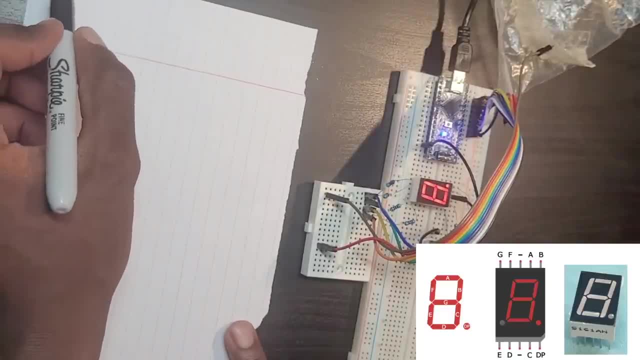 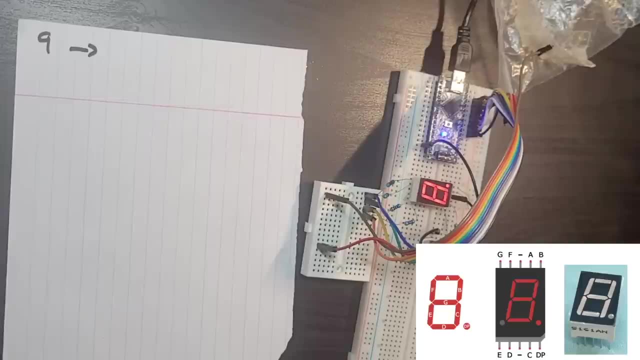 okay, so for nine, what do i need? what do i need to turn on for nine? let me just keep writing this: for nine, what do i need to turn on? i need to turn on a, b, g, c, d. so i need to turn on a, b, c. 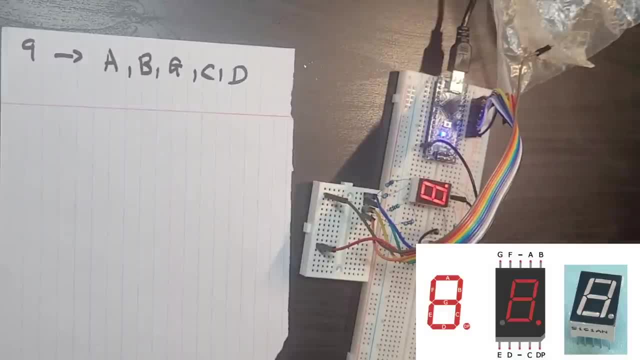 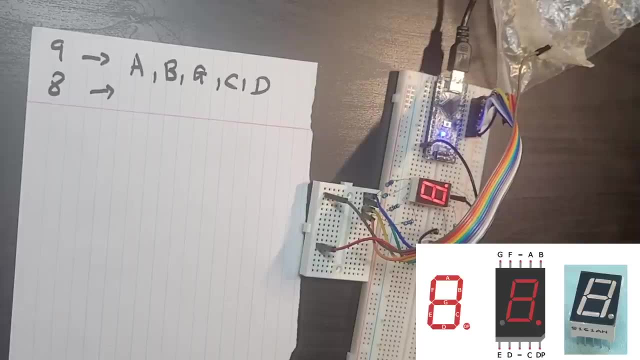 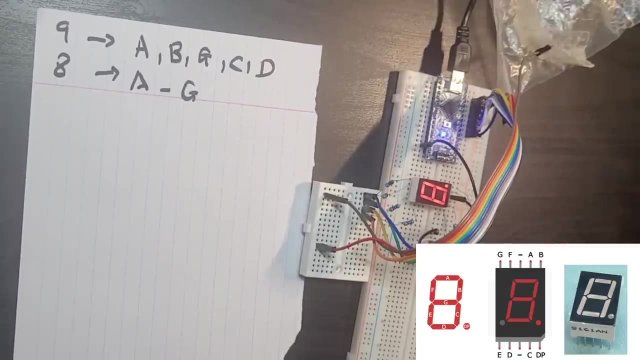 d, g, c and d. let me just make sure again: a, b, g, c, d. all right for eight. what do i need to turn on for eight? i need to turn on everything. everything from what? from a to g. i'm going to turn on all of. 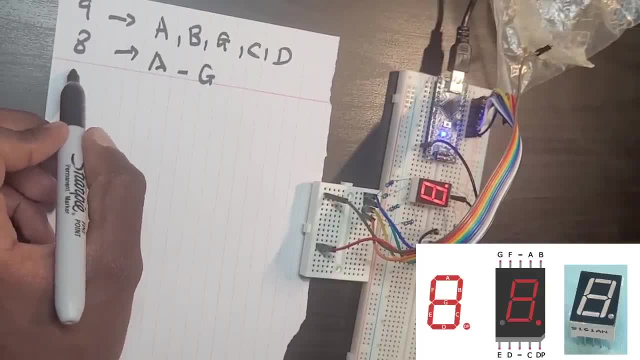 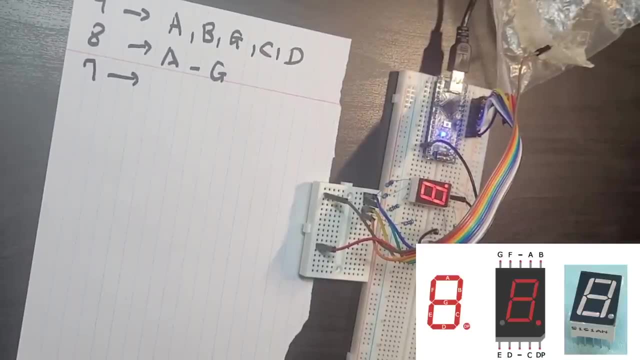 it. i can add the decimal point, but i don't need to. all right, so for um, seven, right here, what do i need to turn on? i need to turn on a, b, c, d, all right, so for eight. what do i need to turn on when the equalizer goes from a to e to c, a. 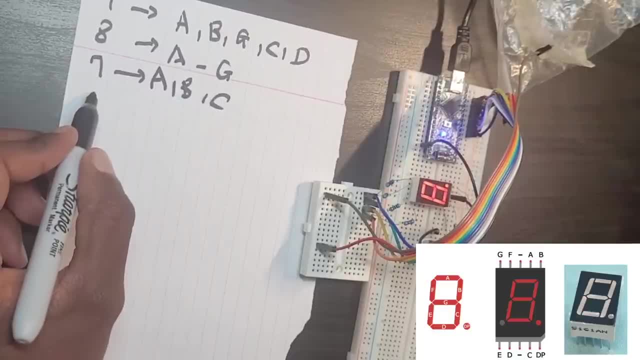 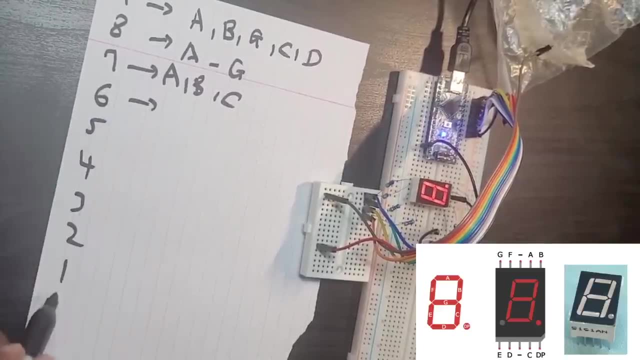 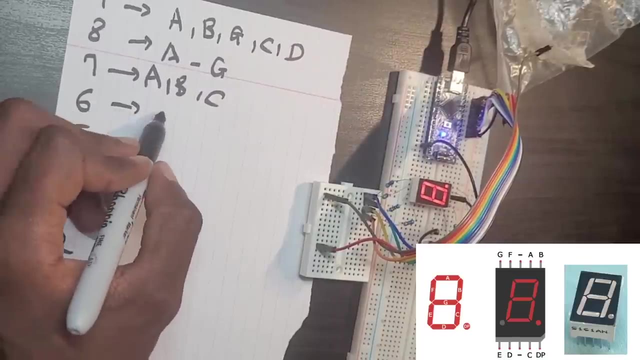 d, c, a, ne, a, b, c and so forth. i'll add them up to the number ace and seven, eight, mom, whatever you want, all right. so for eight, let's call him. let's say a, b, cy, ac or a, c, cal, c, ya, a, b, c. for seven, then six, the number is down forced, it's easier that way. one then end at zero. okay for six. what do i need to turn on? a, f, g, e, f, j, if i did six? 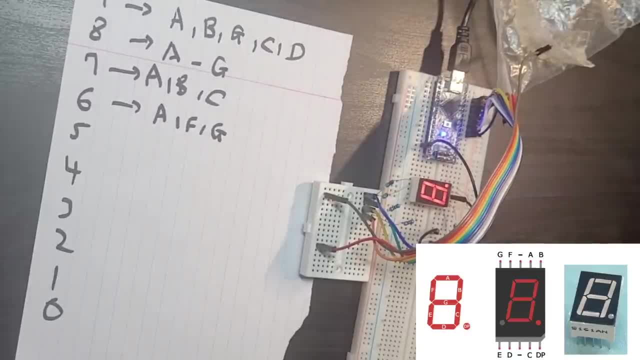 let me first go a, f g c, a, f g a, then e, c d. let me just play around with it first. so if im not sure, if i'm just playing with e and e c d and then e and e will beicion Copis alersa. 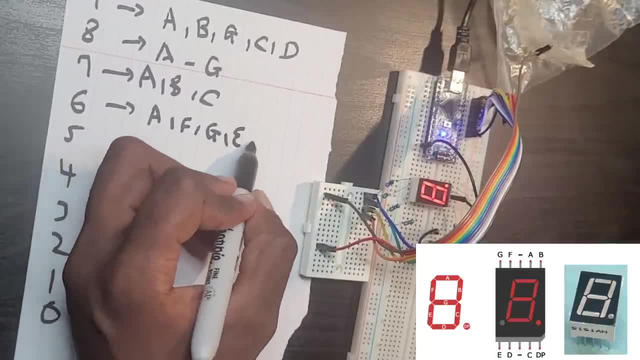 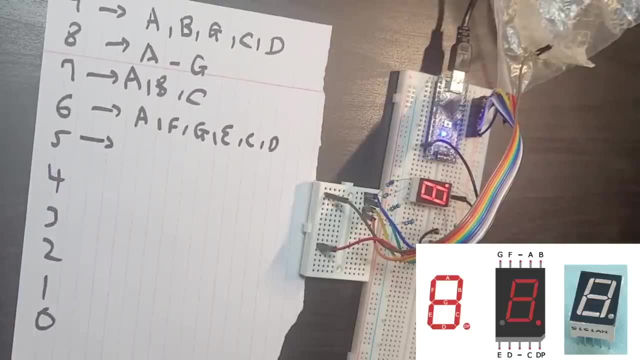 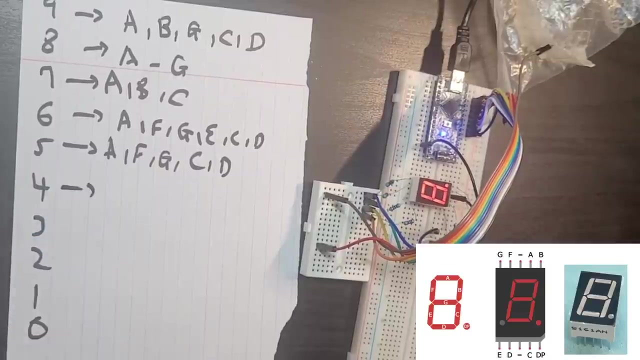 A, F, G and then E, C, D, E, C, D. basically turn on everything except for B, then go to number five. what do I need to turn on? I need to turn on A, F, G, A, F, G, A, F, G and then C, D, just write that down. C D for number four. what do I need to turn on for? 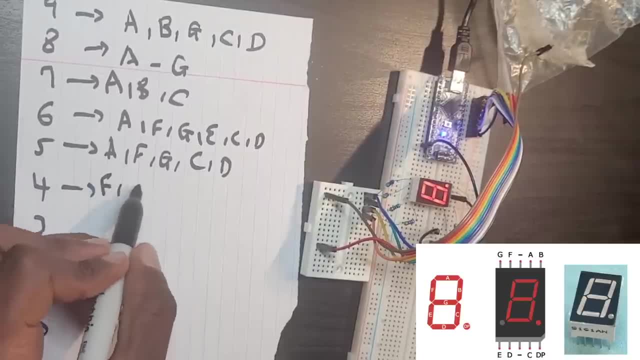 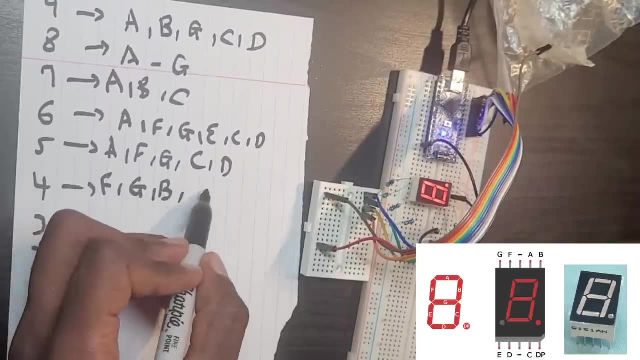 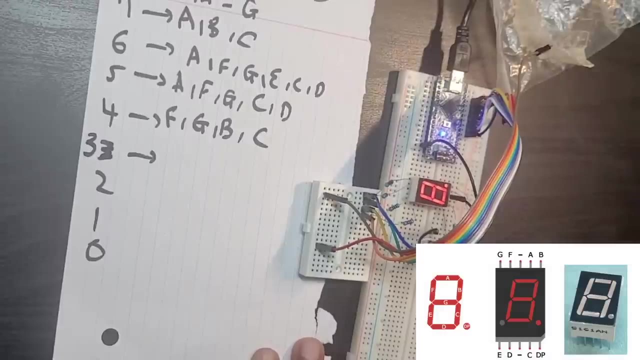 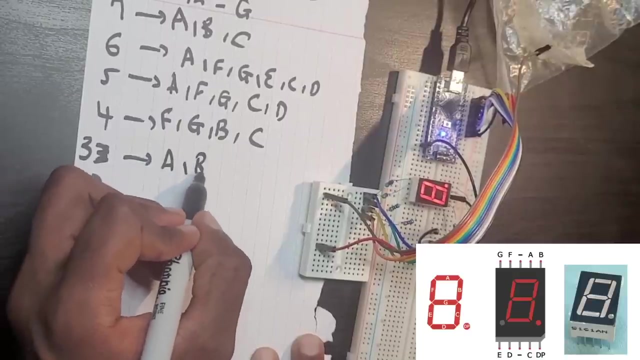 number four. I need to turn on F G B. just write that down: F G, B. and then I need to turn on what? C? that's what I need to turn on: C. then for number three. I did not write down number three properly. there we go for number three. what do I need to turn on? A, B, G, A, B, G and. 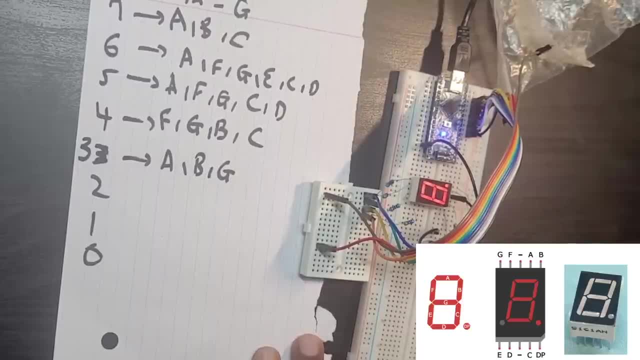 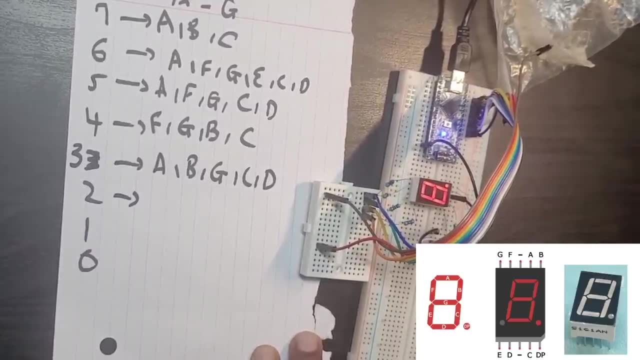 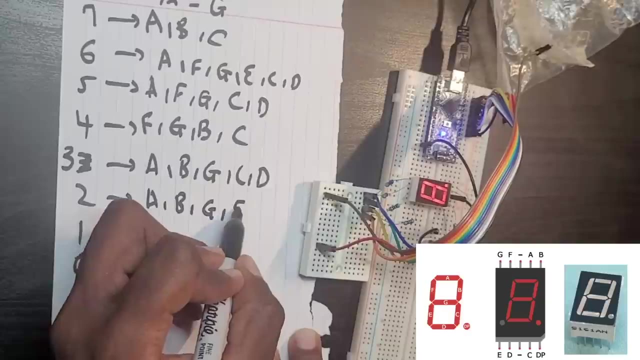 then C and D. let me just check it again: A, B, G, C and D. yeah, C and D for number two. what do I need to turn on? I need to turn on A, B, G, E, A, B, basically G, and then an E, A, B, G, E and then finally a D. 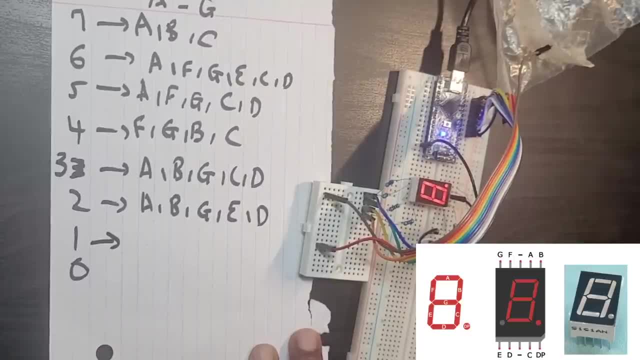 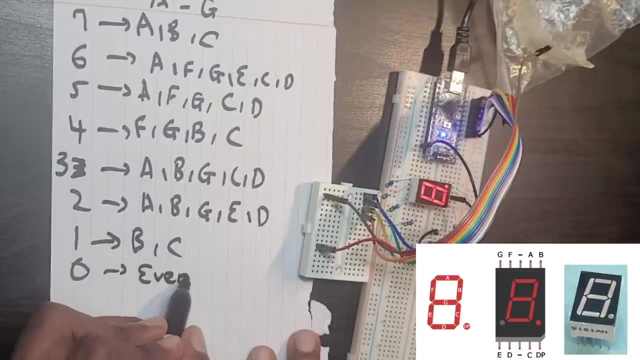 okay, for number one, what do I need to turn on? I think number one is the easiest one. I can either turn on B, C or or fe. i'm just gonna go to pc, i'm gonna choose pc. there you go. and then, finally, for number zero, we're going to turn on everything except for g. let me just write that down: everything. 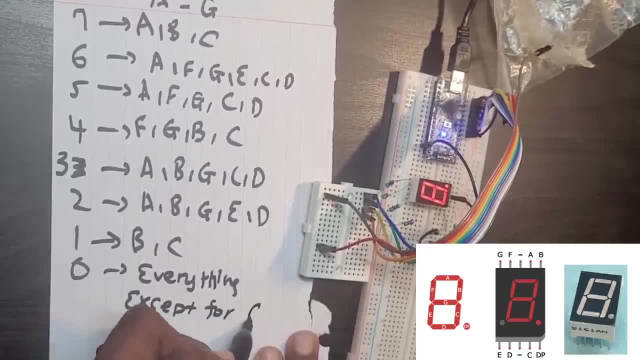 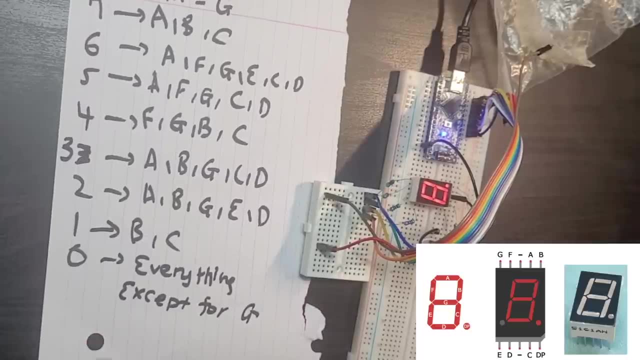 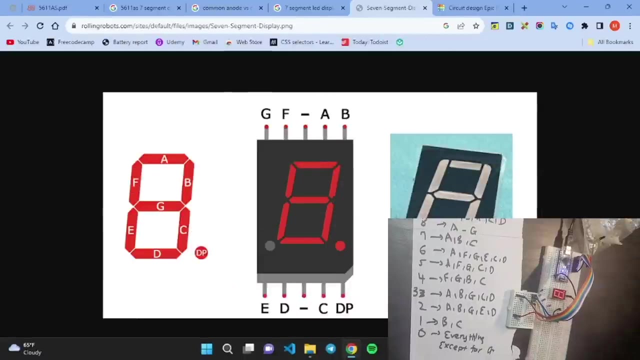 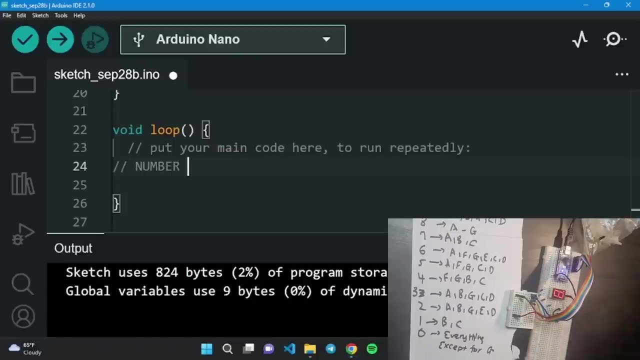 everything except for, except for g. okay, there we go. okay, so that's all i need to turn on. so let me start turning this on. okay, so let's go back again to our arduino code, arduino ide. and now let's start. let me just write here number, what number? 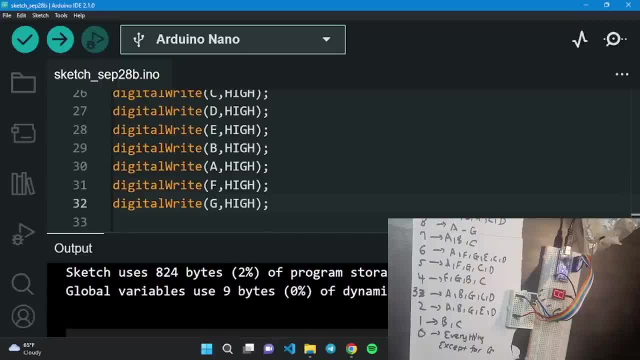 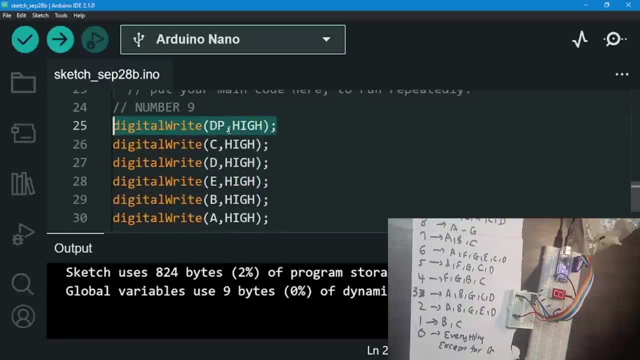 nine for number nine. what do i need to turn on again? i'm going to copy paste this again. what i'm going to need to turn on is what the decimal point. i can remove the decimal point. i don't need to turn it on. i can, i can. 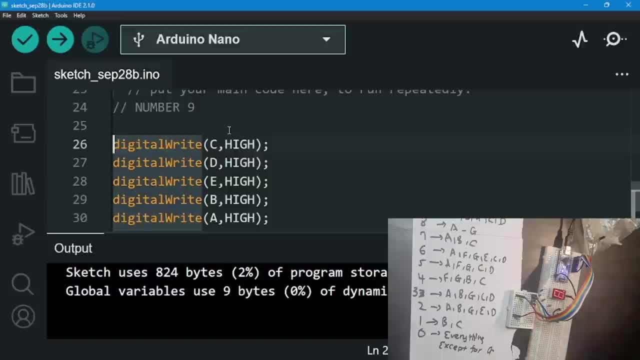 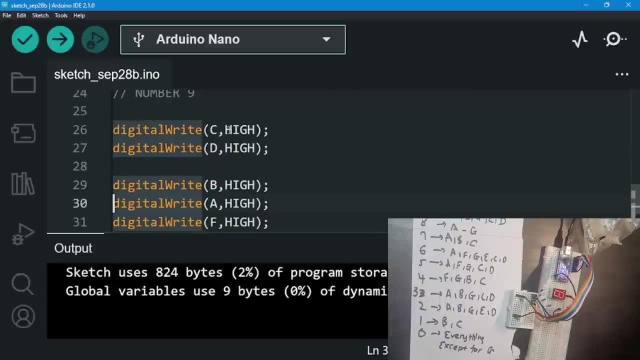 you decimal point. okay, what do i need to turn on? a, b, g and c and d. so i'm going to leave c, i'm going to leave e. i'm going to leave. i'm not going to leave e. i'm going to leave b and a. that's it. 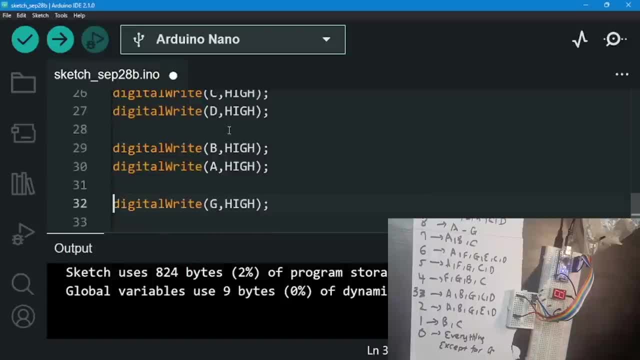 that's all i need to turn on, except for what? g. okay, there we go. so i'm going to remove f and g. there you go. so this is for walk for number nine. how about for number eight? just write down number eight, number eight for number eight. what do i need to turn on again? paste this first. 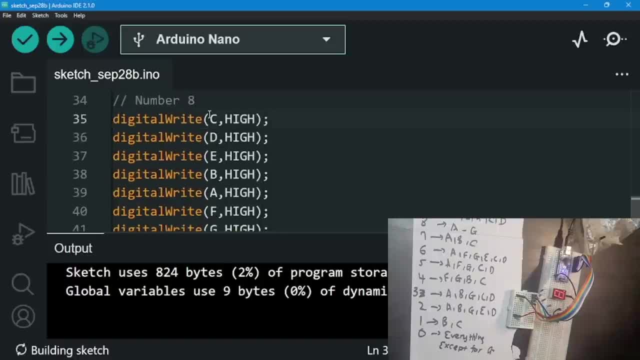 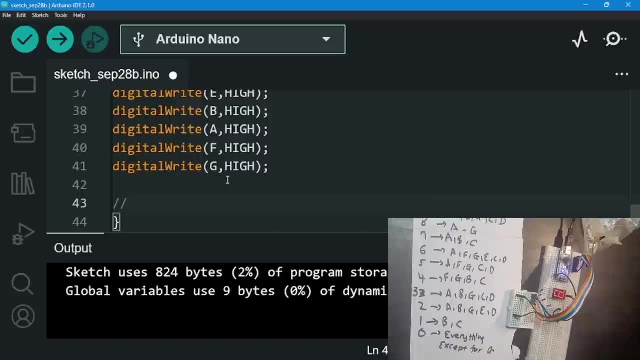 and then I'm gonna need to remove decimal point and then I'm gonna turn on everything from A to G, So I'm not gonna touch anything. Everything's from A to G's already ready. There we go. And then for number seven. okay. 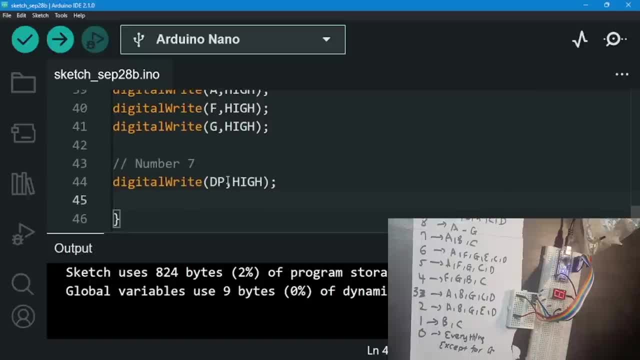 What do I need to turn on for number seven? A, B and then C? okay, A B and then C. Okay for number seven. let me just let me go to my clipboard right here, Control-Z. 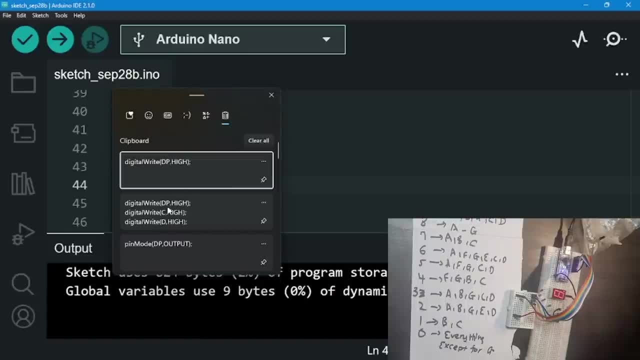 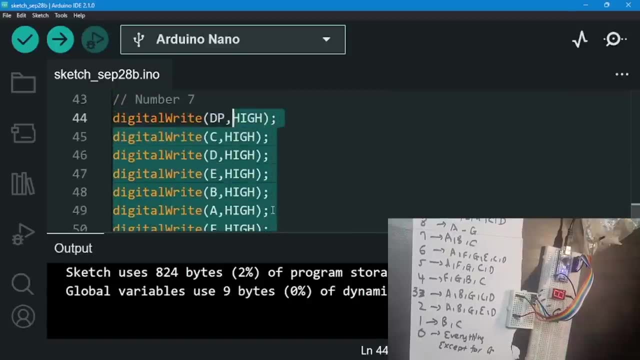 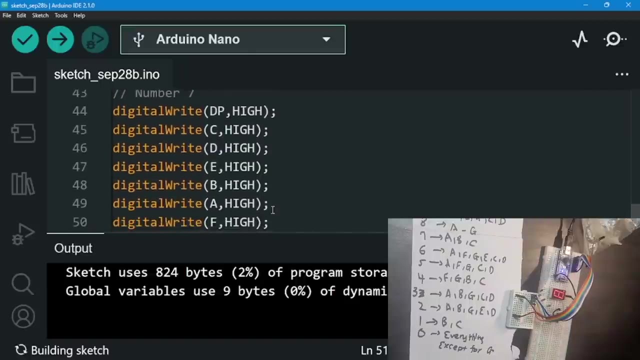 I'm just gonna go here and just say Windows and V. I'm just going to my clipboard. I forgot about this. I accidentally, just I accidentally. there we go Again, copy this again and just turn it off. I can paste it. 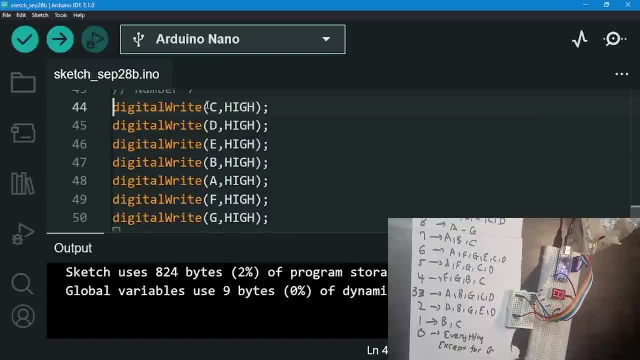 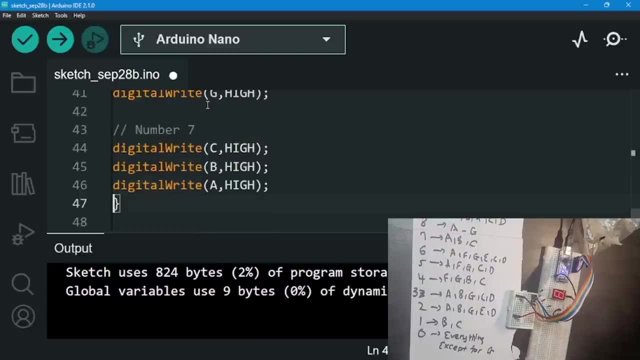 There we go. So now, what I'm gonna need to turn off decimal point. and then, what do I need to turn off Everything except for A, B, C, Okay, so I'm gonna turn this off, turn this off, turn this off. 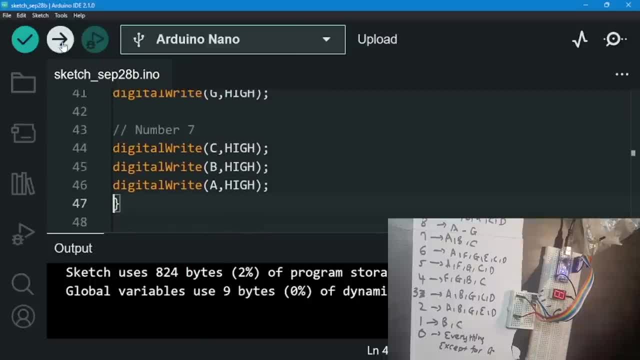 And this off. So lemme just check how my code goes until here. Lemme just check it. So let's just try and upload it, Let's compile it And then it's done uploading. What did I do wrong right here? 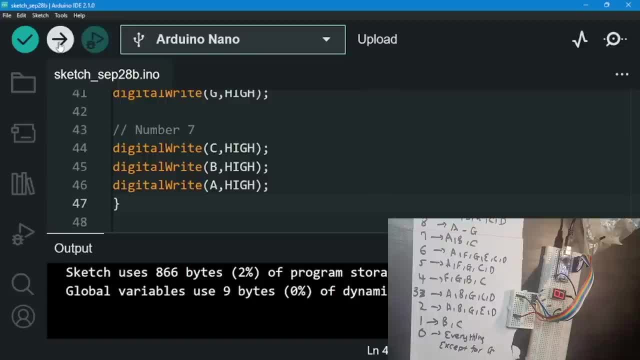 It doesn't even look like any number Right here. it doesn't even look like a number. Looks like a six, an inverted nine. from my perspective For you guys, the most likely looks like six, which is way wrong, Just so wrong. 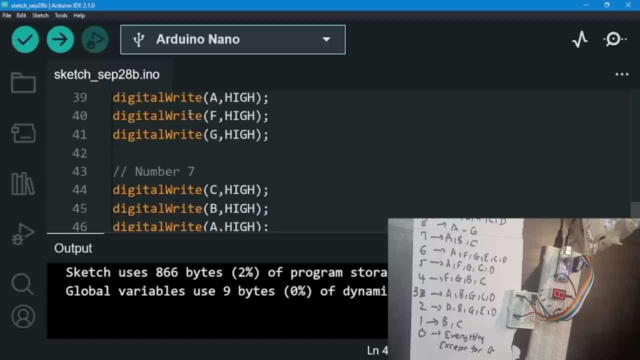 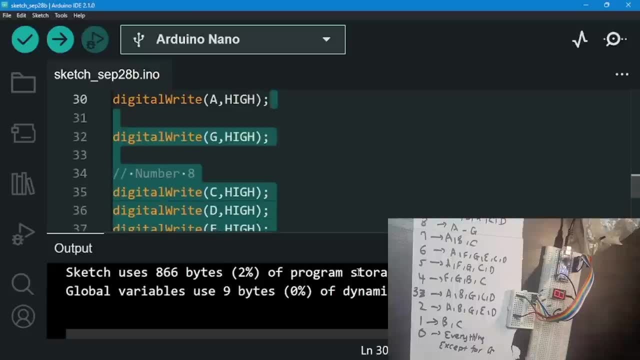 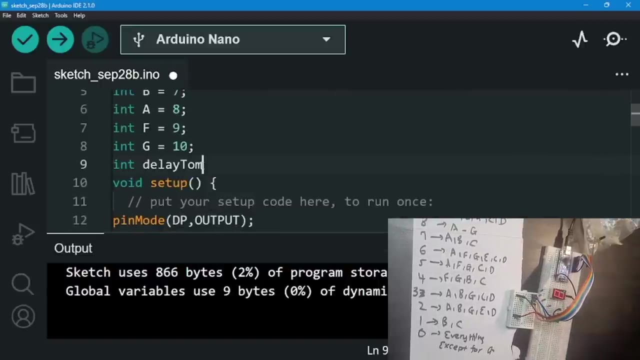 here. hmm, there is a problem now. okay, so what I need to do right here is what? give it a delay, forgot a delay? oh so let me skip the variable right here. let me say delay time time. we're gonna set it to second. I want it every second, so I. 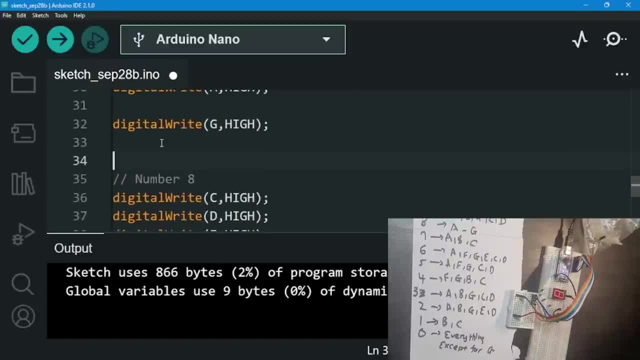 wanted to decrease every second. so I'm going to give it a delay between every number. that's what I need to do. so let's see how it progress. so delay time: skip that. keep writing delay time. for every number delay, I'm gonna give it a delay of. 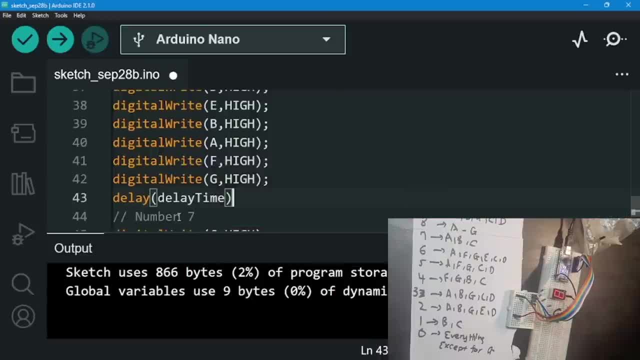 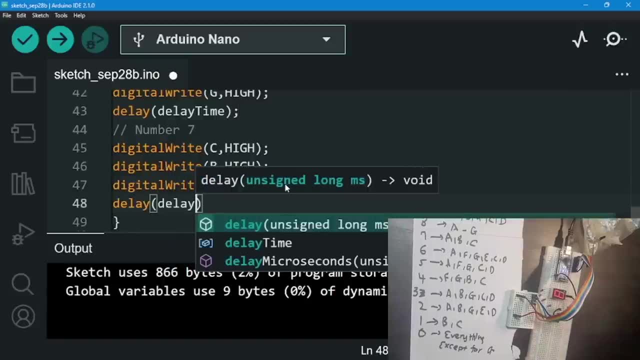 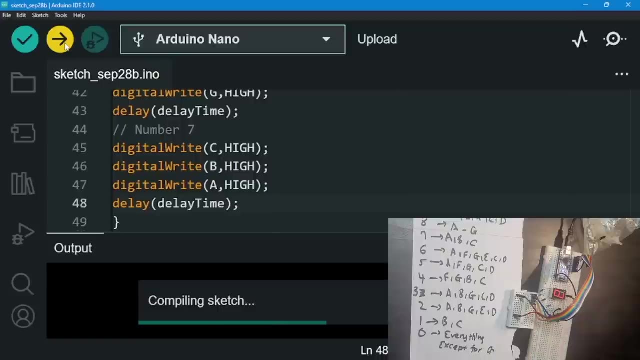 what delay time, delay time. there you go, end it with a semicolon, at the very end, put a semicolon and then finally give this to a delay time. delay of what a delay time, delay time, time. and then let's set it up. okay, now let's see what happens. I gave all of 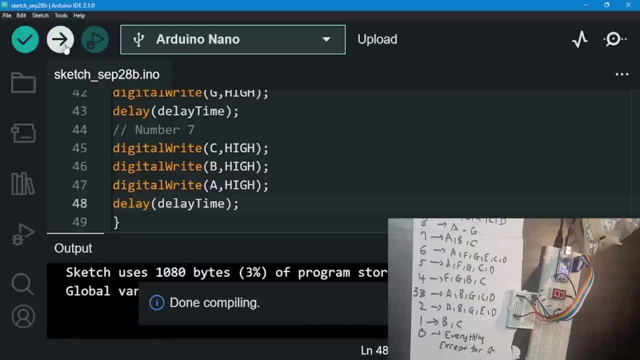 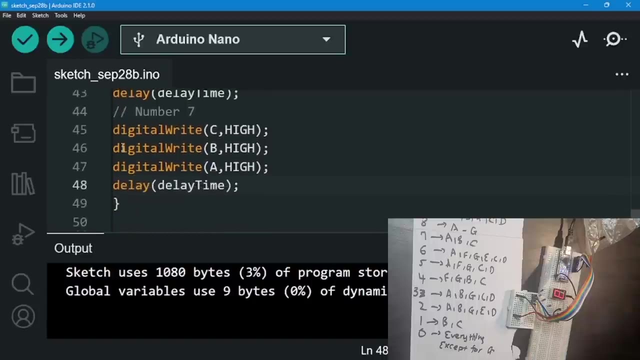 them, delete them. let's just see what happens again. I'm just trying to go again. that seems so wrong, doesn't it? it seems so wrong. well, and the one thing I want to say, I want to repeat this places and again: yes, I've just changed everything in here again and copy this here, and I've set. 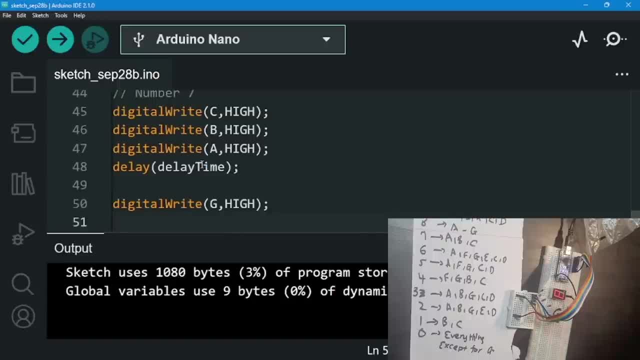 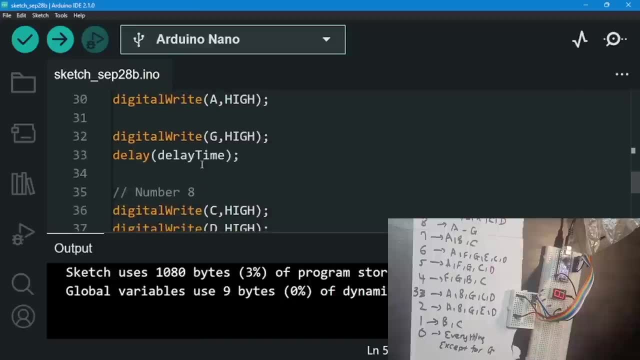 it to to zero. what can we have done wrong? okay, here we go, and so if we start down, that's okay, interesting. so in order to do this, we have to give it a delay. what could we have possibly done wrong? let me try to again turn on everything. 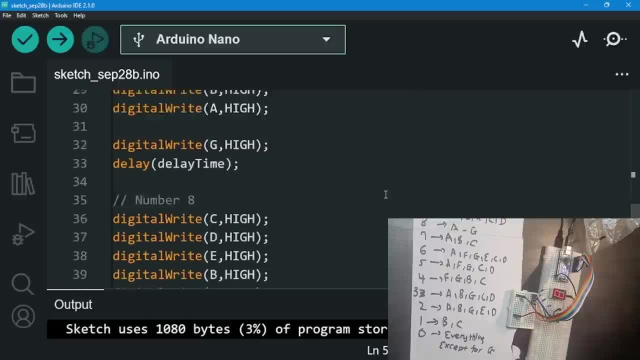 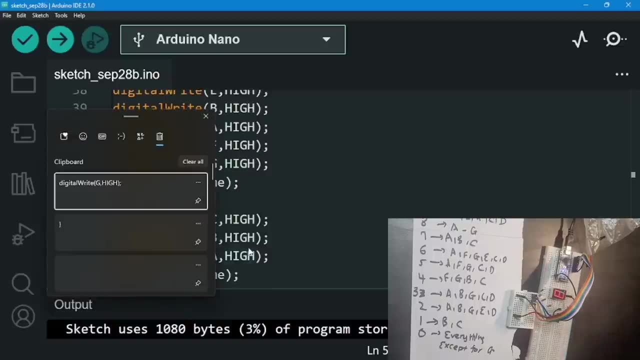 down here. what did i do wrong? i think everything seems fine, so let me just see if everything's even well coiled up properly, so that everything is even what it's. even the resistors might be a problem. so let me just check the resistors at the problem here. let me try to find my. 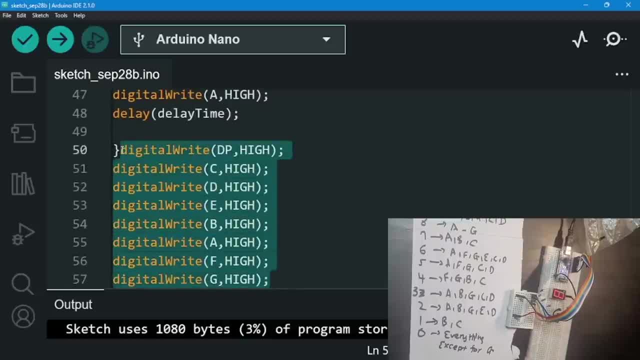 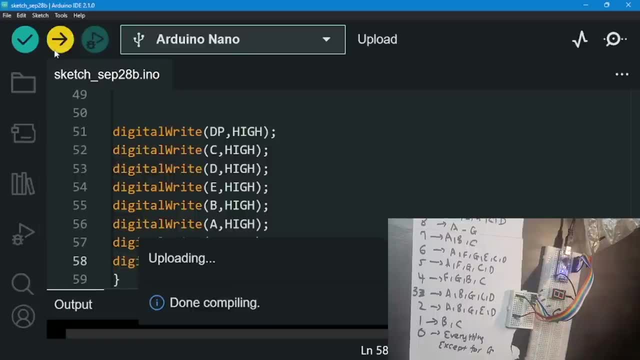 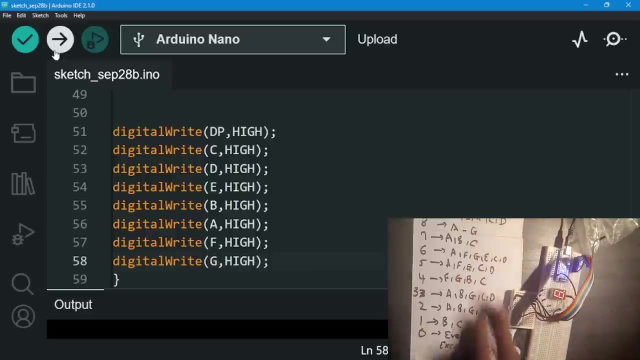 there we go. finally, i'm going to set it to all of it too high, so we can actually see it ourselves. is it the resistors that are making a problem right here again, or are they the eyes? is it or is it our code? let me just check. i'd be our resistors. let me just turn off the light. so 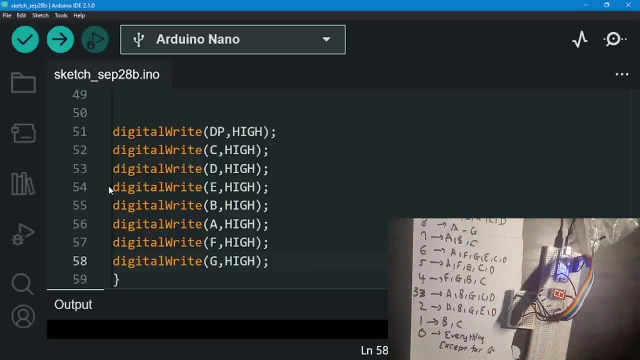 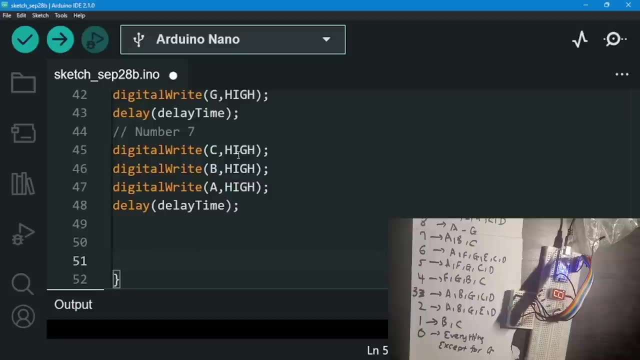 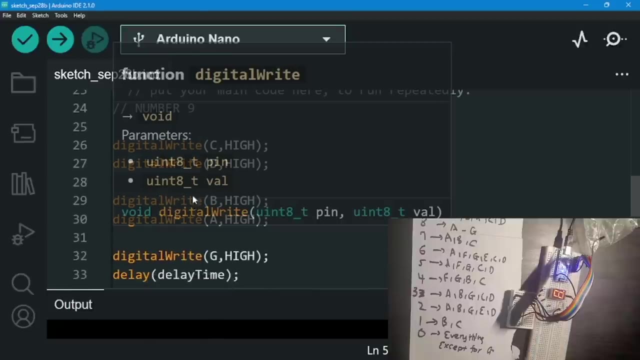 you can see way better. okay, when i finally turned it to what off, to why everything seems fine. what could we have done wrong then? hmm, okay, we don't even see nine at first. we see nine, first number nine. did we see nine properly? so we got c, d, b, a and g. let me give the delay time even. let's give it a more. 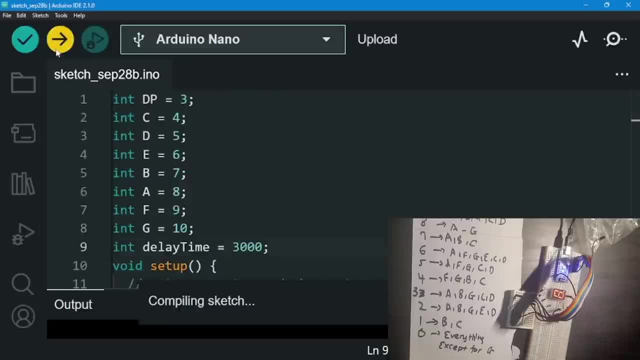 time. let me see three seconds, every three seconds. why is that so? because i want to see where the error arises. okay, where the error starts. so let me look here. even the nine's not correct, and then i change the number, okay. so what could have done wrong? here is what. 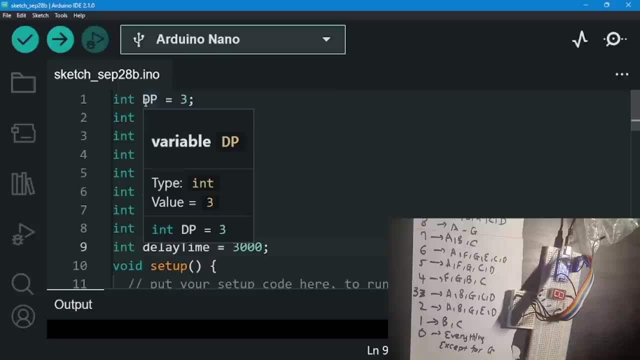 what i believe we could have done wrong here is naming it while we're naming the variables. so again, i made a mistake. it happens, as i said again, but right now i can again check it- what relatively. that's the best part of it. you can check it what relatively. so let me go over here. 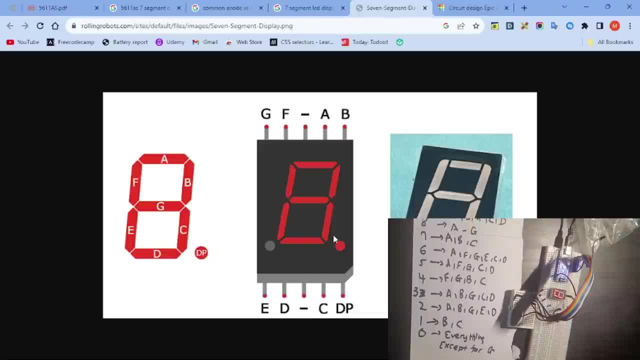 and let me bring my diagram again. i went through the another mistake. again it happens, but right here there's a black wire the blacks connect to. what to pin to? what does the black indicate? the black indicates what decimal point. right, yeah, the black is the one that's going to the closest one. 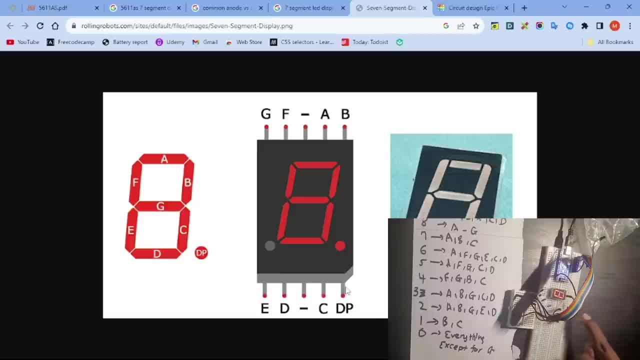 i'm correct? yes, the rooster here. and then it's connected to this one. so it's connected the closest one. so the black goes what to the one? to the decimal point, am i correct? it goes to what? to the decimal point? all right, let's connect decimal point. what did i give it? it's pin what it's pin one. it's the first pin, it's. 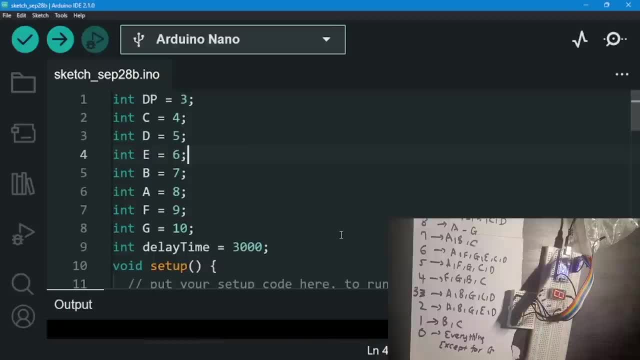 pin one. let's start from pin three, so this should be correct. okay, this should be correct, and then let's go to the white one. the y1 seems to be connected to the other one. let me just again keep checking on the wires. just gonna keep on doing that. 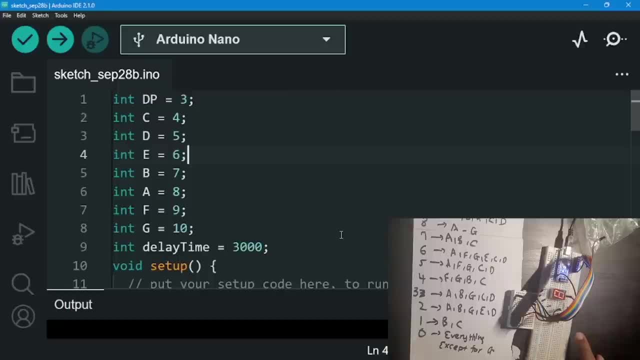 okay, i see the problem. i think i see the problem right here. okay, no, actually i don't. everything seems correct. all right, oh yeah, everything seems to be correct. the first is connected to here, the second is there, the third is there, the silver one. the silver is next to the. 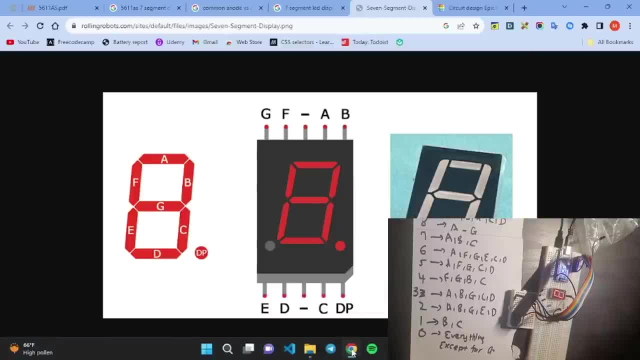 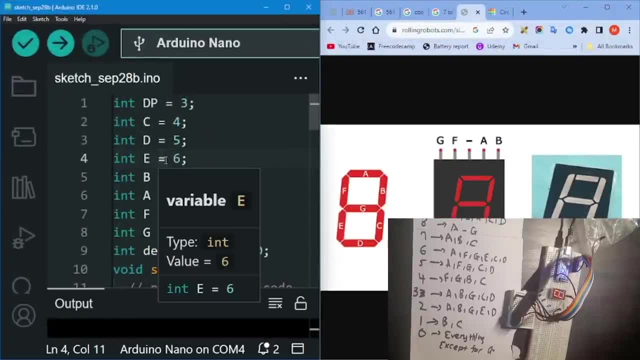 purple, which makes sense. uh, did i get anything wrong? let me just put it side by side again. just put the side by side. okay, that's all i need to do. i'm gonna need to set it up side by side, and there's pin e and there's. 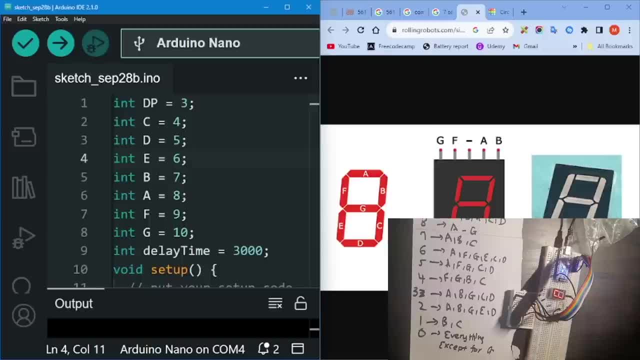 pin d. hmm, what could be our problem? okay, set pin e to what, set it up by number decimal point, and then c, and then d and then e, and then wait after e. i said to e, okay, there we go, i'm correct, i set it to e and then i start to the other side. what could be the problem right here? what could be the problem? 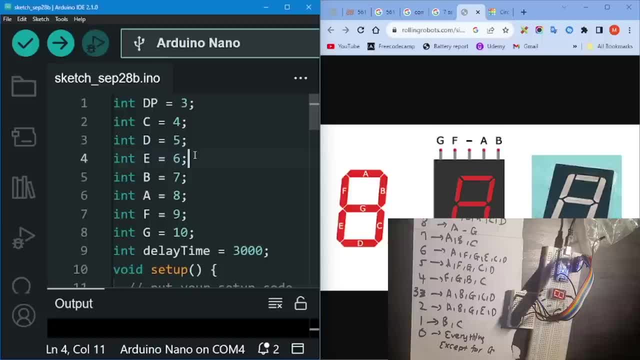 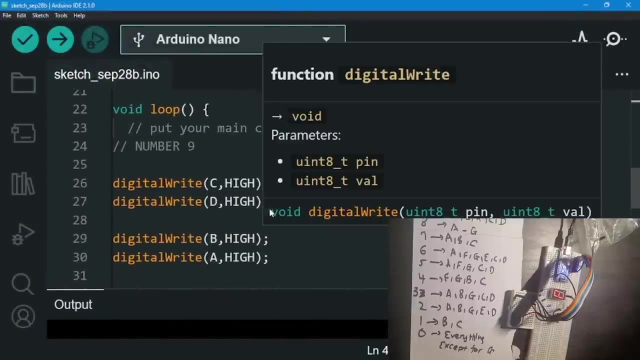 so i want this to finally light up as what as a nine, so one problem that i did, one problem there is. let me show you one problem there is right. here is what one problem that there is is that i keep forgetting to do what, i keep to give it low. 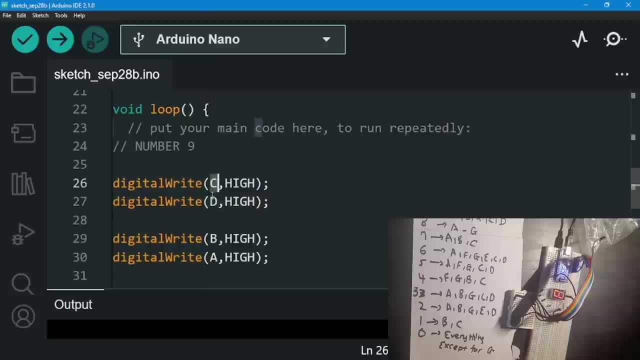 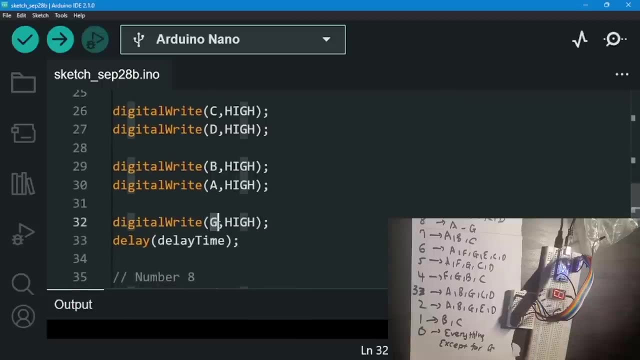 right here. what happens is: look, c and d already set to high. okay, when we're going to number nine, c, d, b are set to high. as i said, you're gonna be set to high. and then, when it comes to number seven, and again g set to high two. okay, wait, is g supposed to be set to hot? it's not, i forgot. 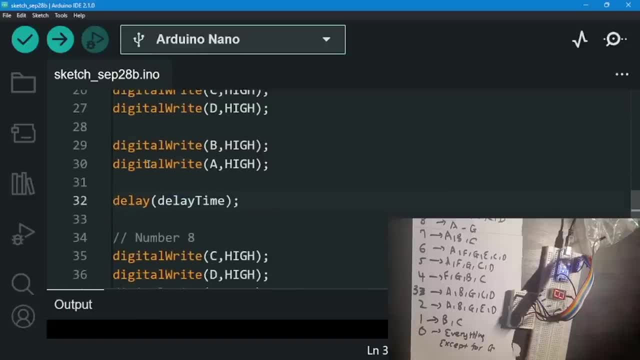 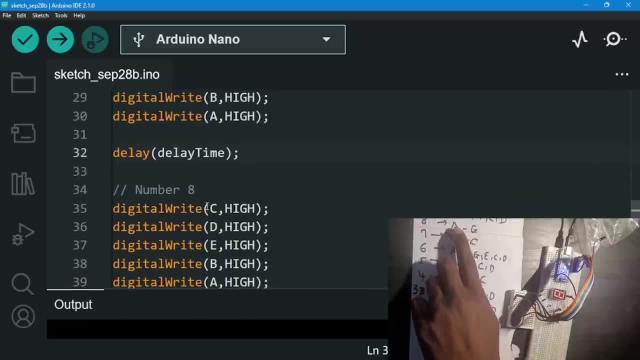 about g right here, let me fix g up. so let's fix g up. and then c: okay, all of it are set to high. okay, a are set to high, and then what happens here is what we only want a to g to set, to be set to high. 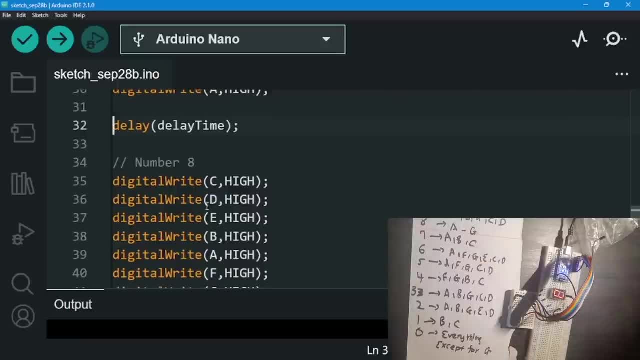 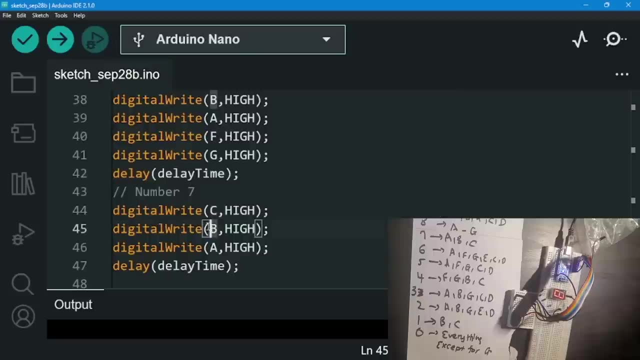 no problem. okay, everything what is set to high, that makes sense. but the problem starts here. what is the problem? right here? can you see the problem? c and then b and then a, can you see it? c- b are the only ones that are supposed to be set to high, but we already set everything up to high. 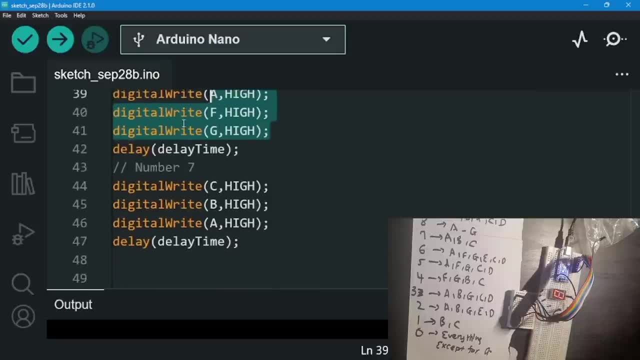 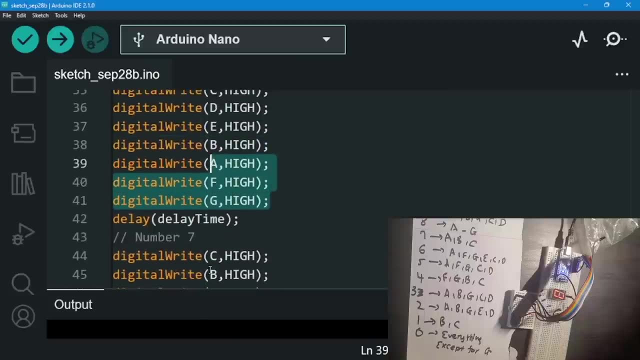 can you see it? we set everything to what to high. this is where the problem starts. okay, so we set everything already up to high, and then we only want to set this to what too high. so we have to what? technically, what do we have to do? we have to turn everything low. before what? 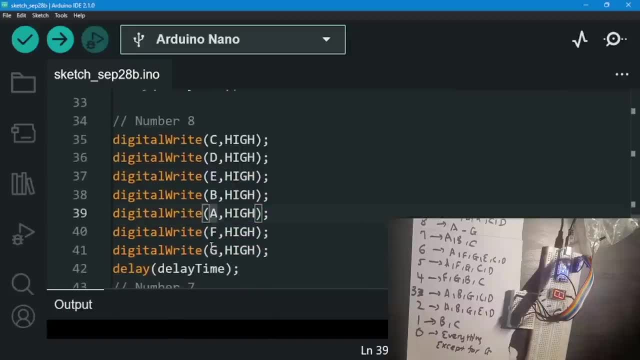 moving into the next one, because right here i said everything from a to g to what to high already, and then when i go right here from c, b and a, i only want them to be set to high. other ones they're going to be set to what to low. well, what i want, like here, is what, what happens, what quite? 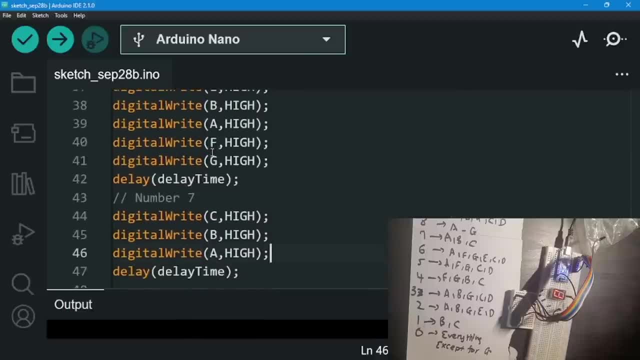 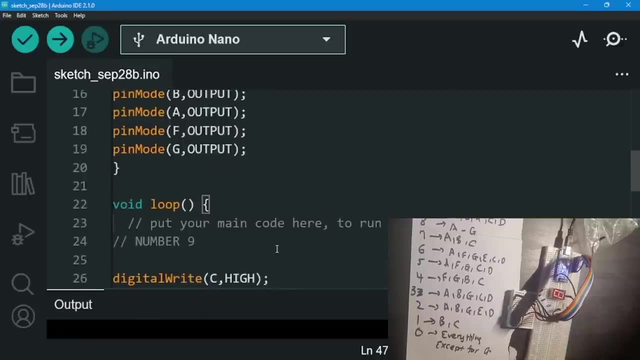 the opposite. okay, so what happens is quite the opposite. so everything is already set to high, and try to set this high again. it doesn't make any difference. that's what's happened, okay, so i need to do is what i need to go over to my code right here again. hopefully, i have everything intact. let 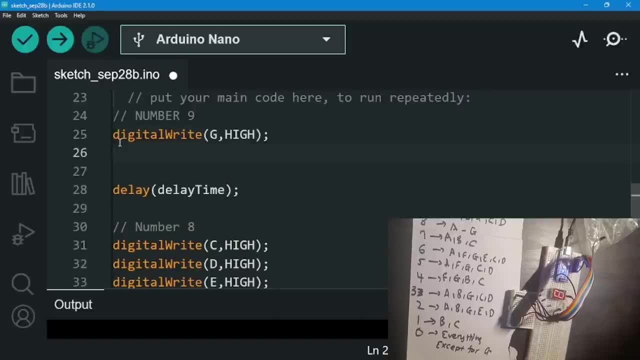 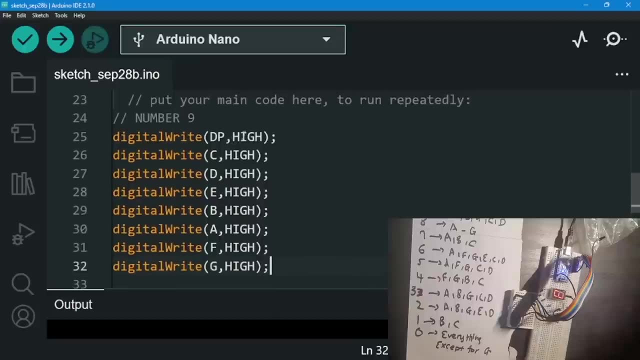 me just get this right, paste this. oh, let me go to my clipboard again. there we go, got everything right. instead of removing them, what i'm going to be doing is what i'm going to be setting them to what to low. okay, the ones that i don't want. i'm going to be setting them to what to low. 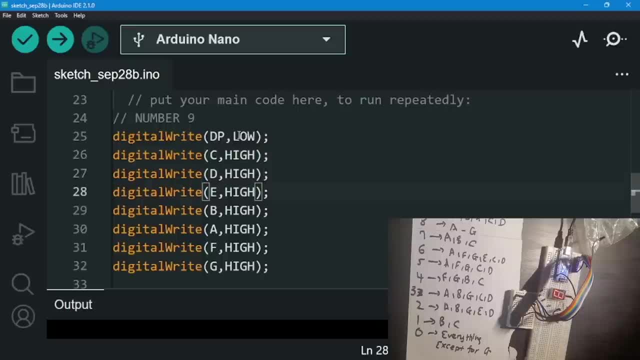 b, g, c, d. so we need c, we need d, we need what we need what. we need e. we don't need e. so what do i do? i set it to low. okay, because it's going to affect the next number that we're going to what? 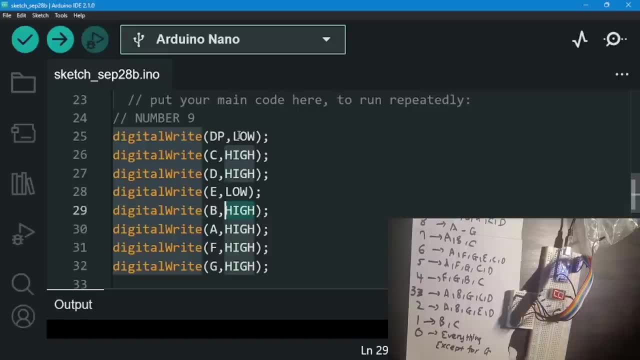 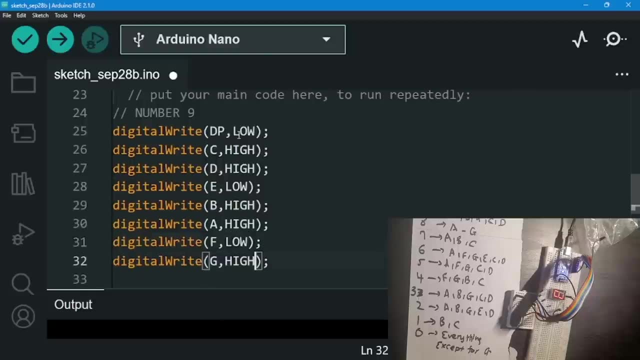 we're going to be touching, so we're going to set this again to high or low. we cannot just remove it. okay, so this was already set to high. okay, it's supposed to be set to high. we're not going to be using f, so we're going to be setting it to low and then our g, okay, 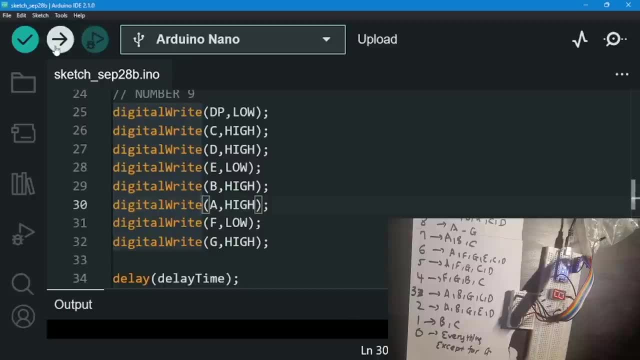 g is supposed to be set to high too. all right, so we're not going to touch it. so let's try to upload it right now. let's even see if we can even see nine as a, as a number. so let's just try to open it. we cannot see what. okay, you see that for the first, for the first seconds. what happens is: 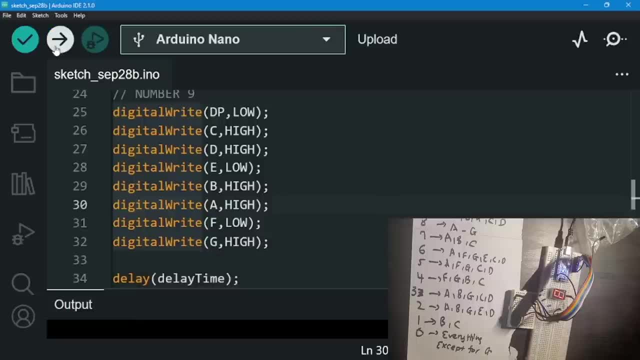 what you don't see, the whole thing light up. we see one, two, three, four, four led segments. light up. how many led segments should be light enough? one, two, three, four, five? let me check my code again. five segments should be set to high: one, two, three, four and five. what could be the problem? i generally don't know what the problem is, so i 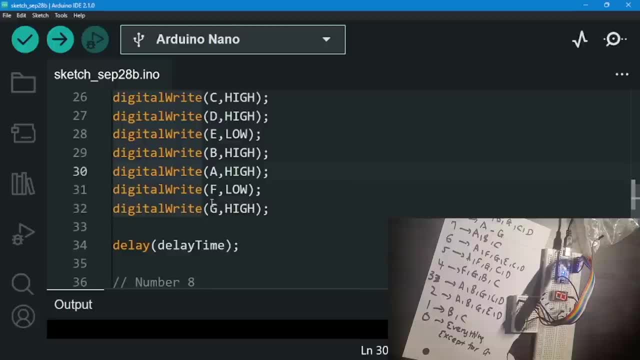 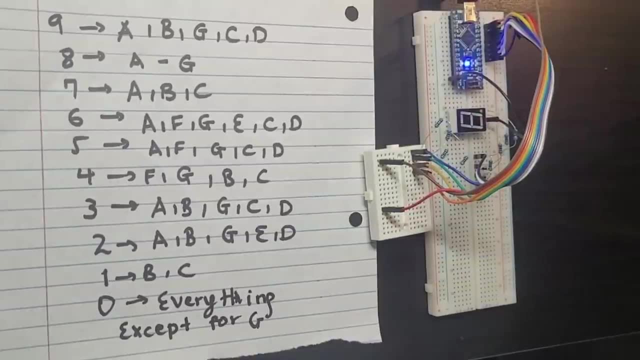 think what i'm going to do right here is, instead of uh, resting, wasting time- is i'm going to try to figure out the problem now myself, and then i'm going to come back here and try to solve it for you, okay, so i was about to re-record the whole section, but uh, i made what. what i made was a very 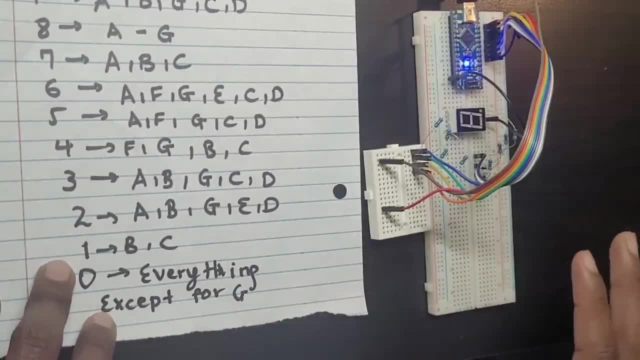 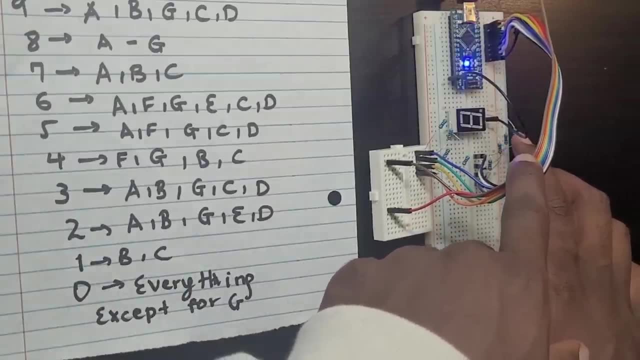 simple. i made two very simple mistakes, the first one being is that the resistors right here are touching- so let me just remove my, move it right here- and these two resistors were touching each other right. so, basically, what happened was when these two resistors touch. 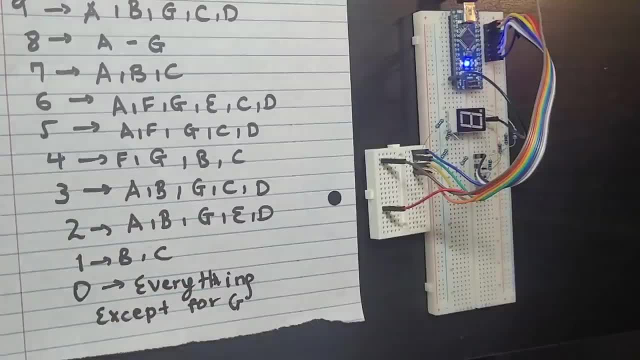 each other. they started to what. they started basically to fuse as if they were just acting as one resistor. so, basically, it was not working on its own. okay, these two resistors. that was the problem that i just made, so there's a good chance that the the code is working for you, um, so right? 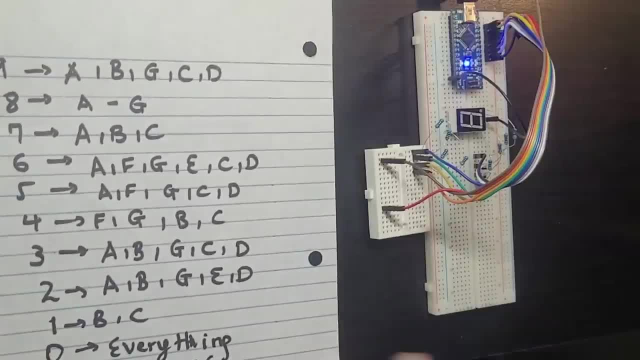 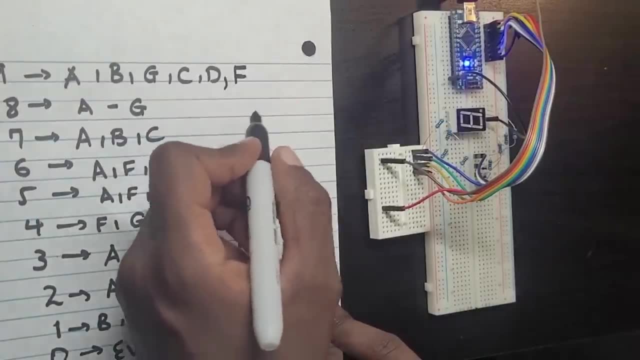 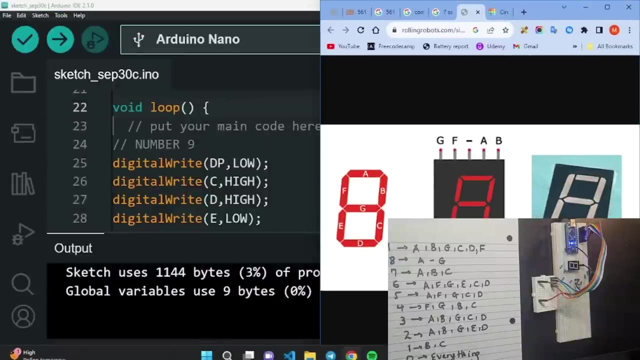 here. that's the first mistake right here, okay. and the second mistake here is when we're using nine, okay, we need to also turn on f. okay, we also need to turn on what f? all right, that's just one thing you have to keep in mind. let me just show you guys where f is. there we go, we need to turn on f. 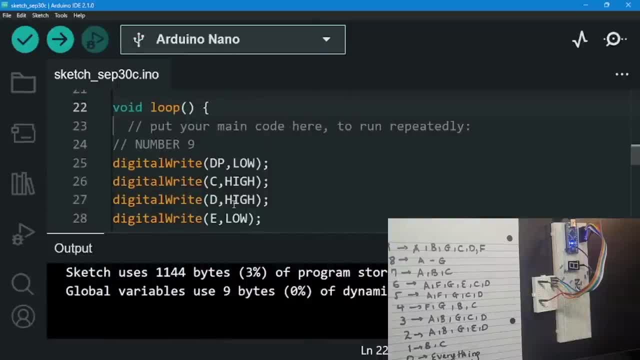 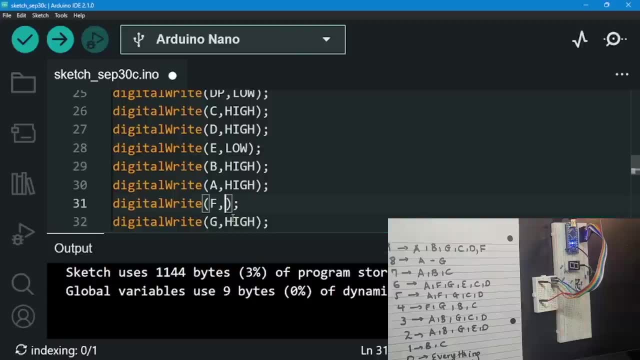 which is supposed to be around here, okay. so, with that in mind, what i should be doing right here is what set this to high. that's our first mistake. solved it. i untangled the resistor right here. i untangled them myself, okay. so it should be working properly right now. i just separated them. 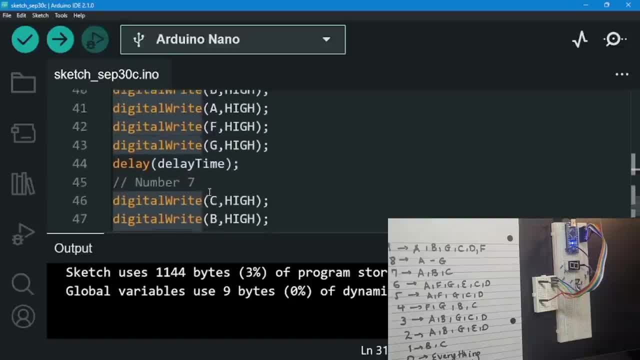 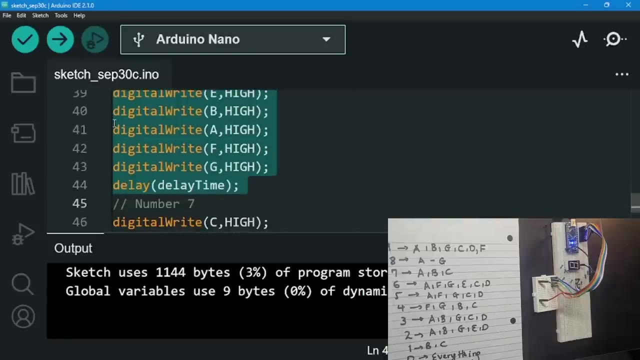 and one thing we need to finally do is what we need to finally write down the whole code of this. obviously i cannot do that for this one. let me just do that. we go here, let me just copy actually number eight, because all of it is set to high. it's going to be easy. you need to copy the whole thing. 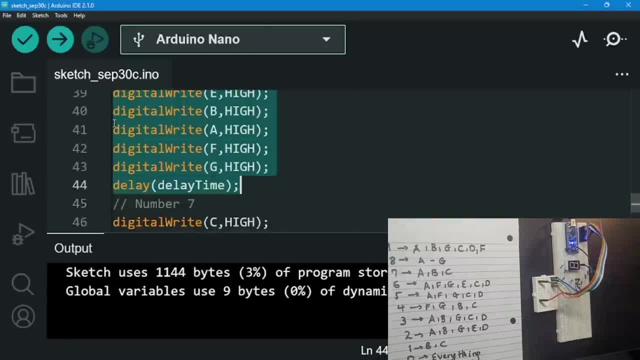 not just part by part. let me just do that, copy that, just paste it here. wait, i, oh, i, i took it off. i deleted number eight. let me just leave it there to copy that, and then i'm going to paste it here, i'm just going to. 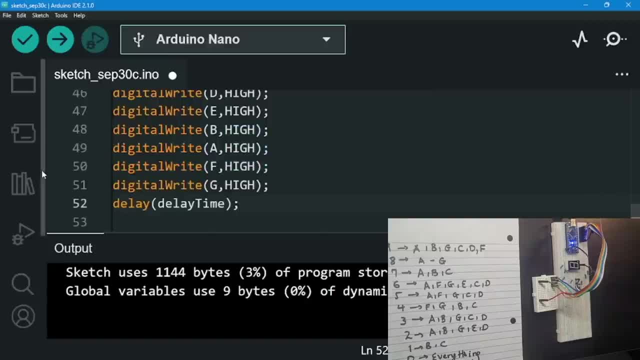 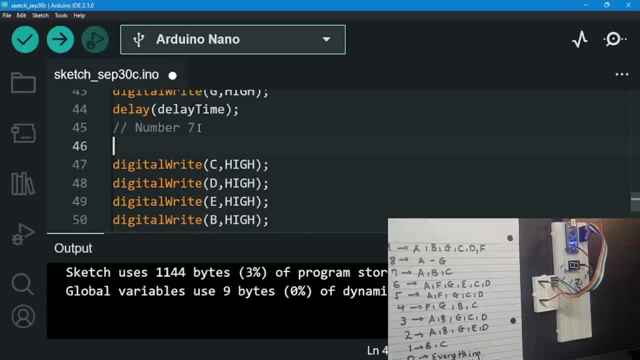 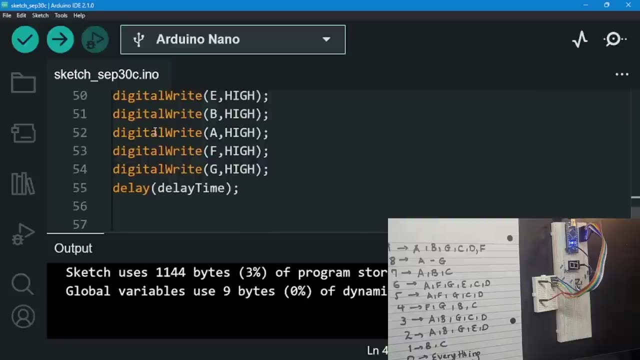 supposed to remove number seven here. all right, there we go. this should be paste. there we go. number seven paste. let me just give it space right here. just you can again have more space. there we go. now what i need to do is: uh, wait, here is what. what is supposed to be set to high abc. so, other than abc, everything is supposed to. 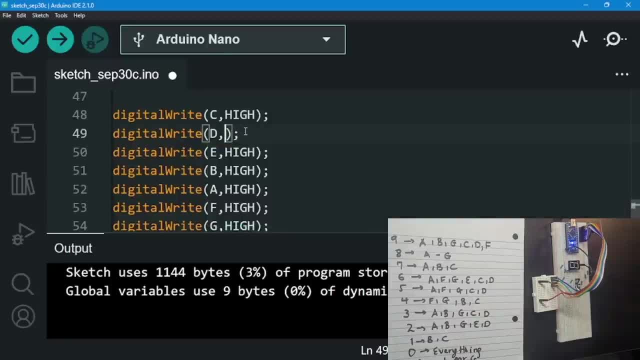 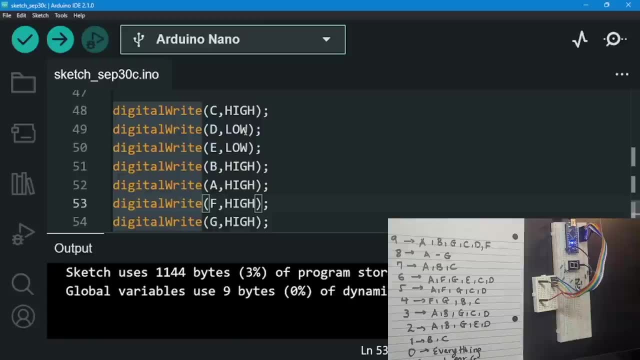 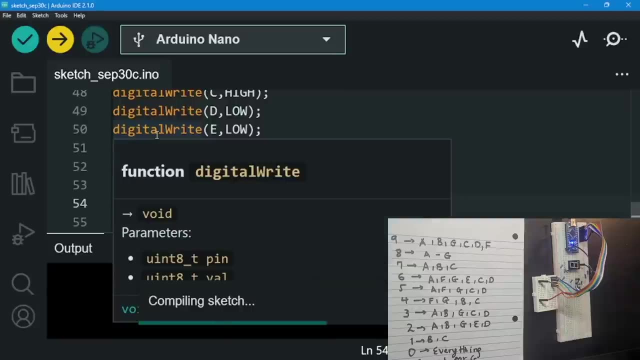 be set to low. just keep on doing that. let me turn on caps lock and there we go, low. abc. i'm supposed to be set to high, so i'm going to leave this one and this one to low and then finally g to low. so now let's just check and upload it. okay, should be compiling and it's working perfectly fine now. 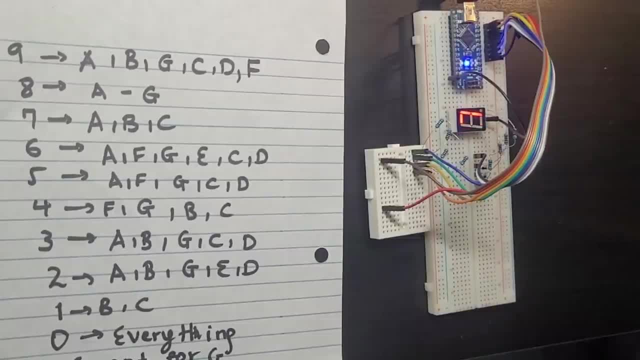 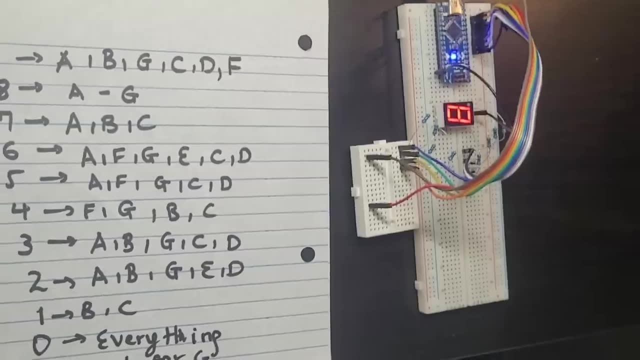 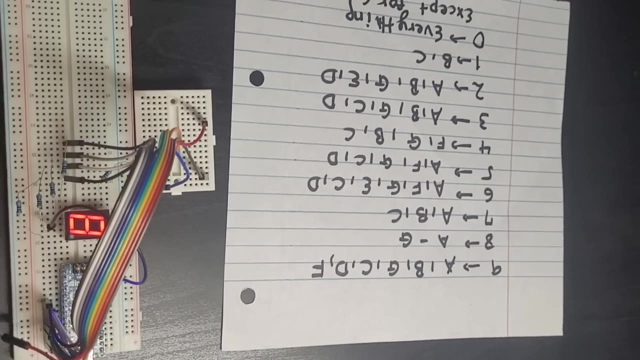 okay, and it's working perfectly fine. it counts to seven, that's good. it goes back to nine, eight, seven. let me just change your angle so you guys can actually see it from the right spot. let me just do that. there we go. let me just put it right here. there we go. let me turn off. 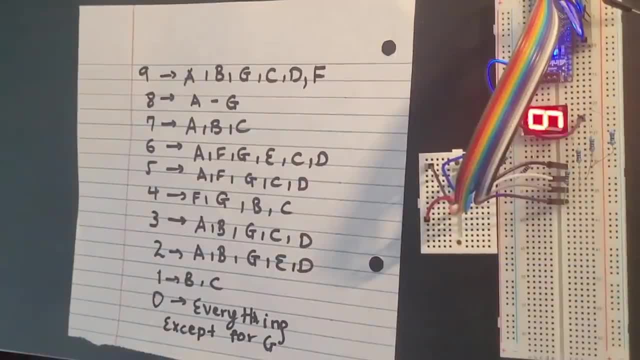 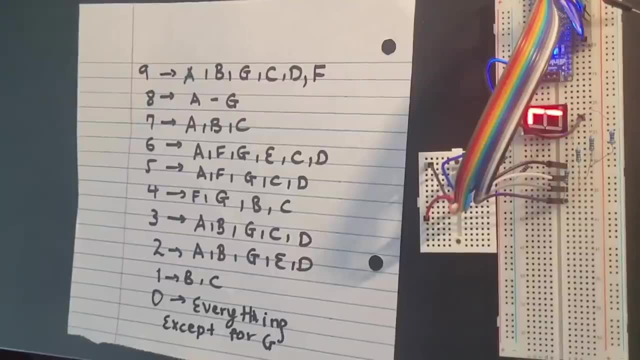 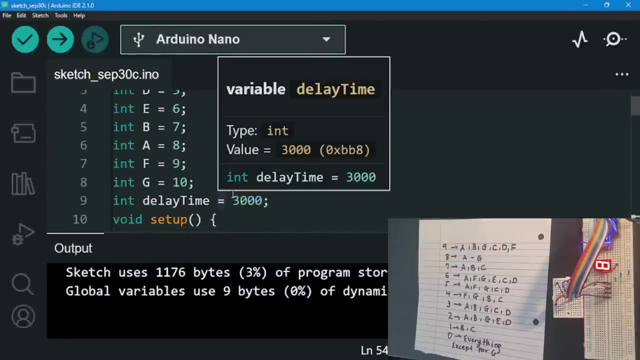 on light so you can see it way better. now you can see it from a good angle. now it's going nine eight seven. okay, the delay time is big, so let me just change it to. it's set to: uh, let me just check it. three thousand milliseconds, basically three seconds. 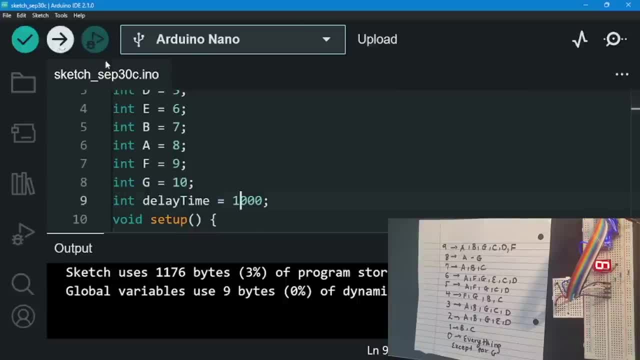 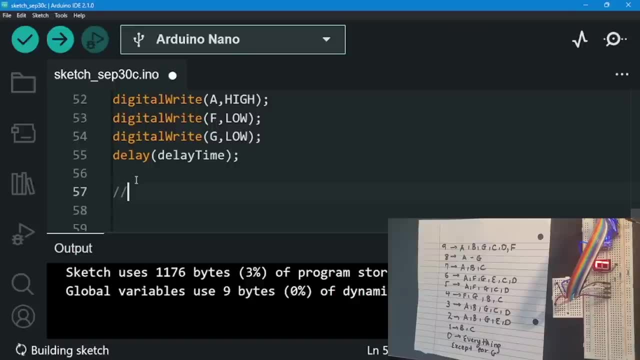 i'm going to set it to what? one thousand milliseconds, basically what a second. okay, so what we're going to do right now is write down the whole number. so let me just write down: we're on number what? number six, number six. what do we need to do for number six again? i'm just 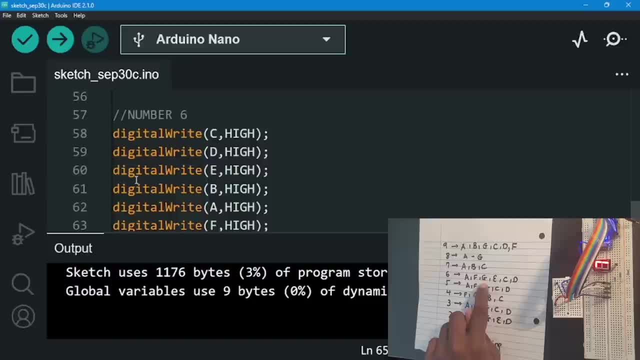 going to paste this code right here for number six: a, f, g, e, c, d need to be turned on. so i'm going to. so basically b needs to be turned off. what else? um, e, e, yeah, basically b needs to be turned off. that's, i think, all that is supposed to be turned off. there we go. so b needs to be what turned off. 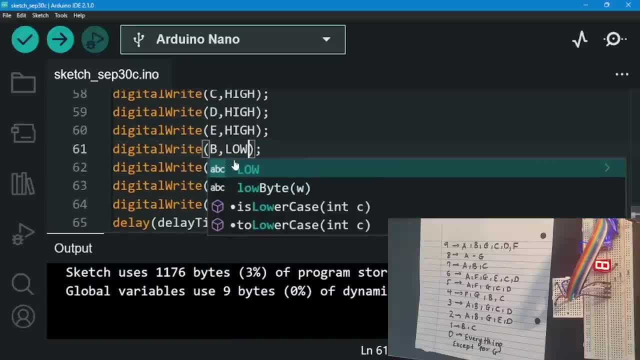 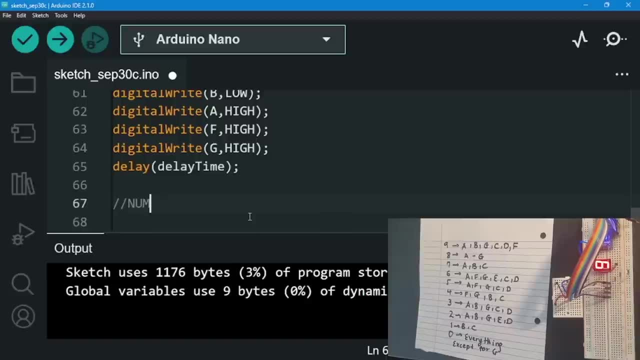 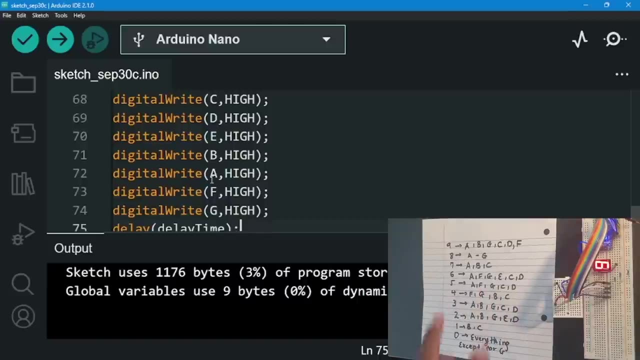 so b set to low for number six. all right now. once we're done with that, i'm just going to set this up to one number, number five. paste the code again. so for this case, one is to be turned off, b, and then e, b and e. 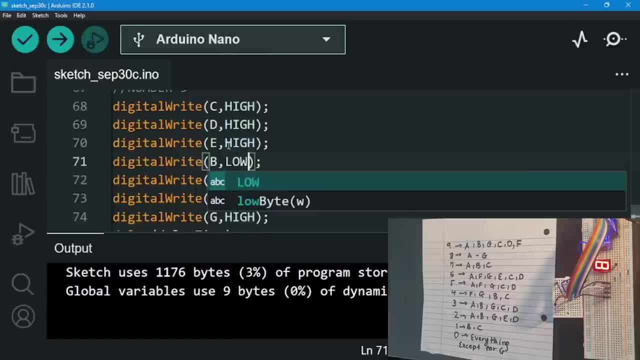 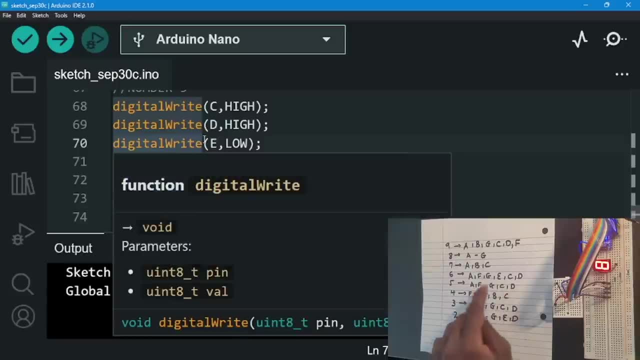 needs to be turned off low. and then for e2 it's going to go low. let me just check it again: a, b, okay, a, a okay. b is going to be turned off because it's not here. then there's c, there's d, e needs to. 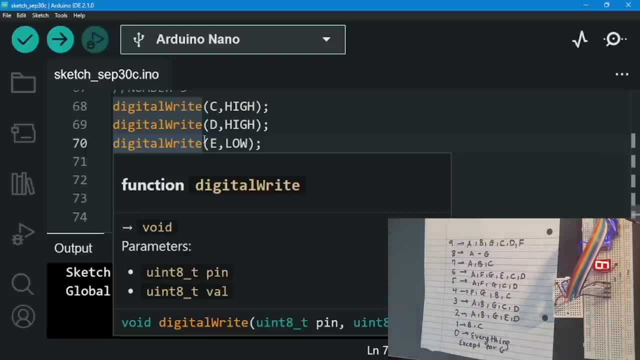 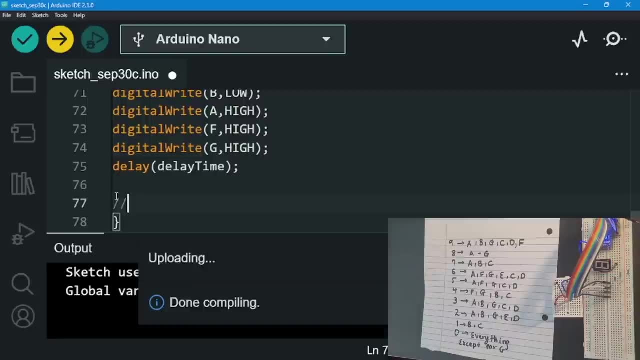 be turned off, and then f, and then there's g, so i'm not going to touch that. so let's just check it out right now. actually, let's upload it. let me write to that time. let me just write down number four. okay, it's going seven, six five. 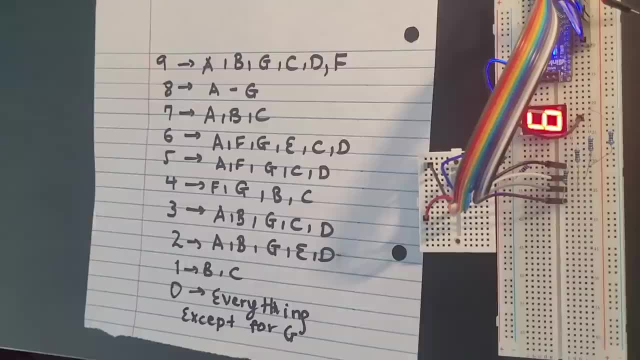 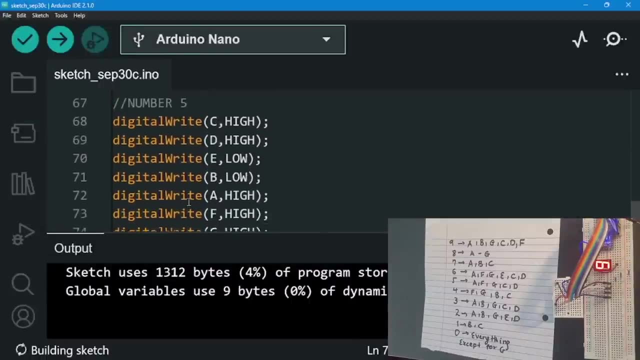 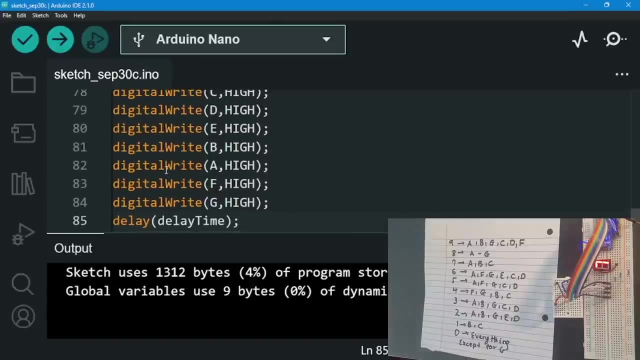 four. okay, okay, let's write down there we go. okay, it went to number five. now let's write down number four. that's all we need to do. let me just write down number four. all right, go to this, though. well, i just need to do is paste the code again. one needs to be turned off right now. a needs to be. 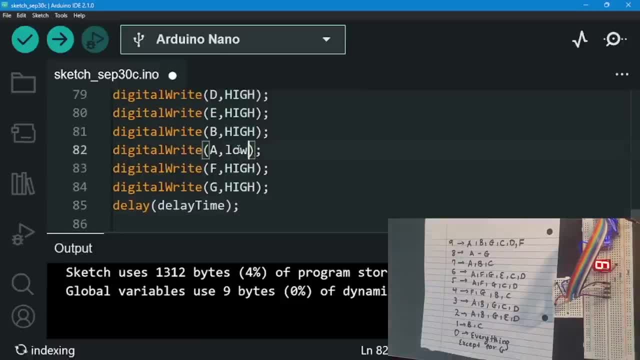 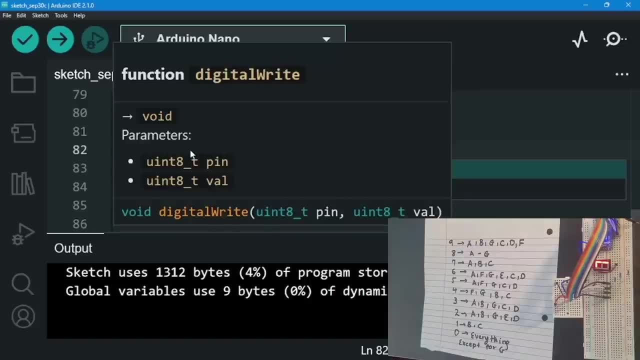 turned off. let me just turn off a first. turn off a. no, i need to turn on caps lock. there we go. turn a off. how about b? b needs to be turned on. c needs to be turned on. d needs to be turned off. let's go to d. 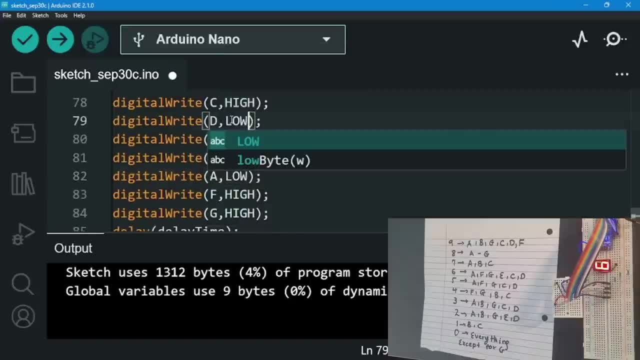 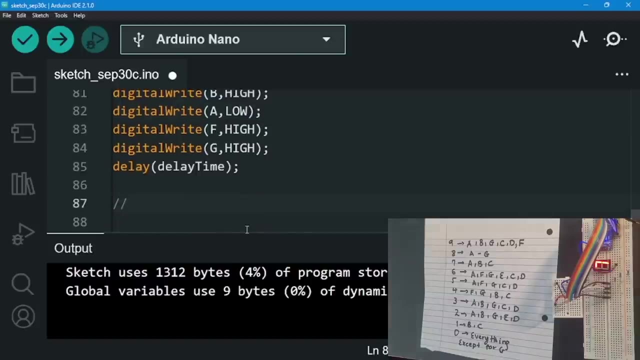 okay, and turn it off. okay. how about e? in this case, e needs to be turned off too. let's go to e. how about f? f needs to be turned on and then g needs to be turned on. so i'm going to leave it like that, okay, and then again keep on doing this for number three. paste that and what needs to be turned on. 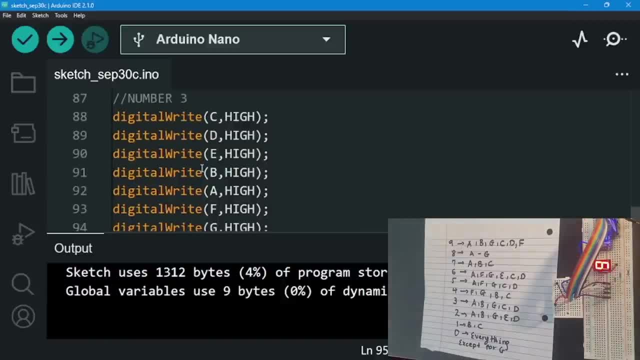 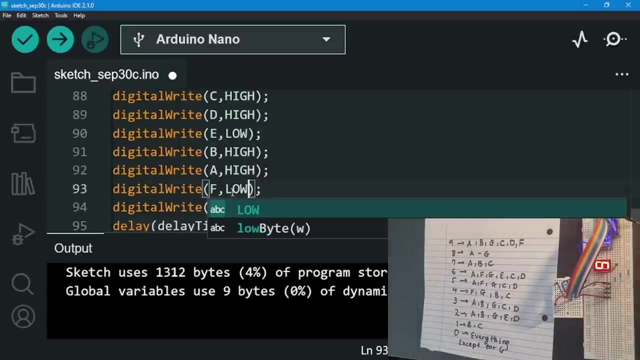 for c: okay, a, b, g and c, d: okay. so basically, e needs to be turned off, okay, d needs to be turned off, e and f needs to be turned off. so let's go to e and f and turn them off. low and f to low- okay. 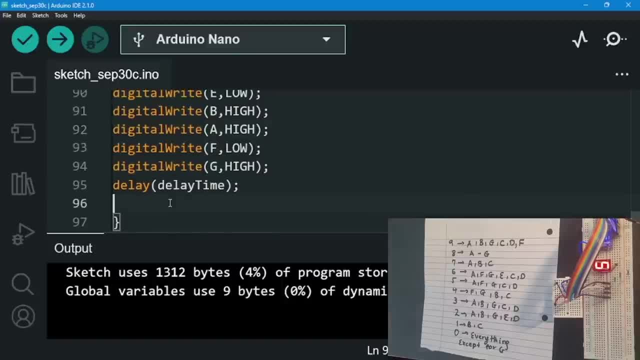 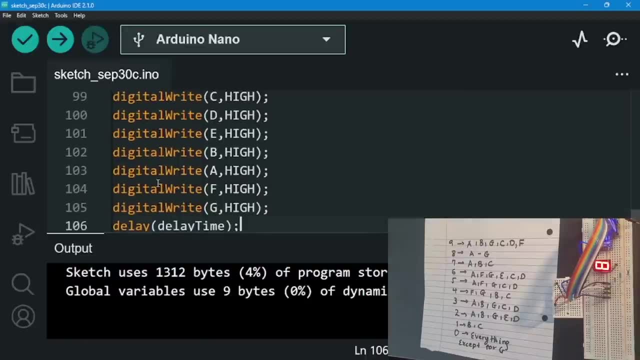 afterwards. let me go to number two. number two paste that for number two, one needs to be turned off c, and then what? uh? d needs to be turned on, so e, then f. okay, so basically what, what c and f needs to be turned off. so let's go to c and f and turn them off. let me turn them to what? to low, okay. 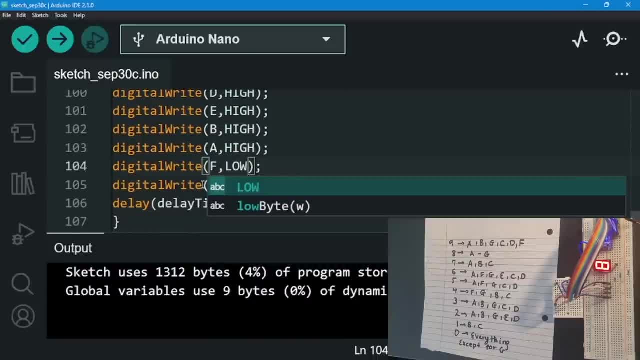 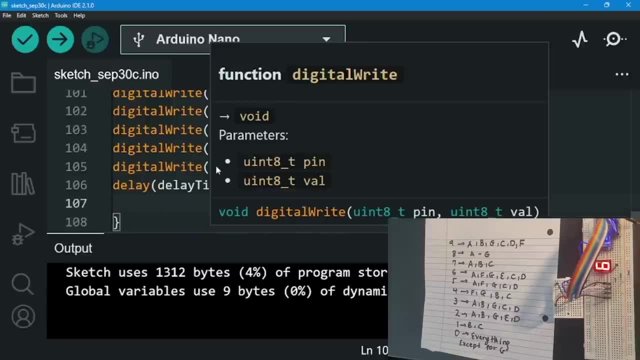 f needs to be turned low again. for those of you are using a cathode pin, you're going to be exactly doing what- the opposite of what i'm doing. if you want to turn off something, obviously what you got to do is what you're: going: to set it to high when you want to. 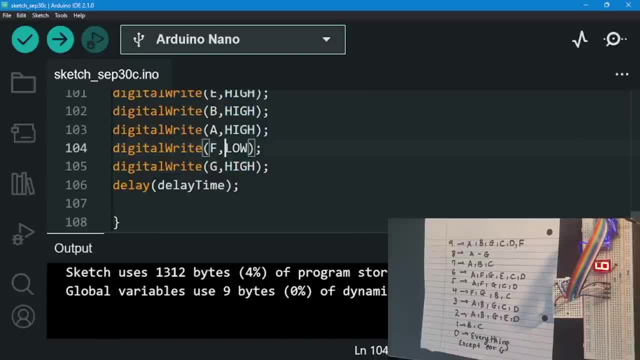 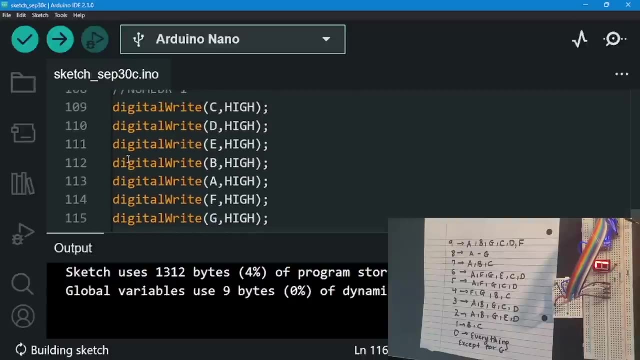 turn off something. we need to want to turn on something. you set it to what? to low. i think you guys know that. all right, let me just keep that in mind and let's move to number one. number one, that's number two, right here. number one: paste that and what do i need to do for number 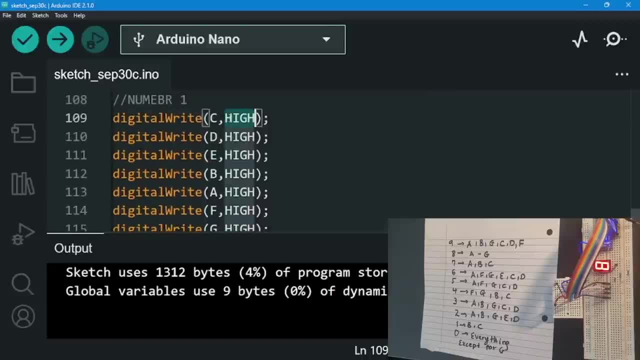 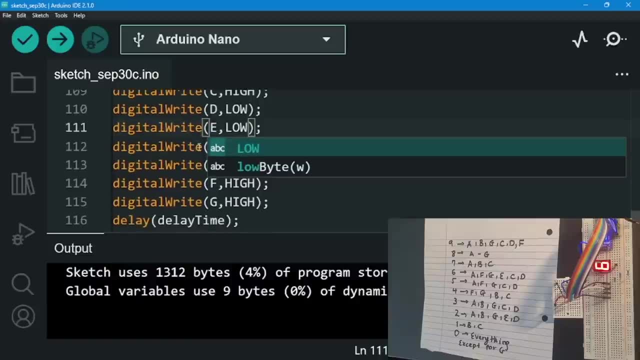 one. only b and c need to be turned on, so most of it is going to be. so what to low a? b and c need to be turned on. just go here. i want e, low b and c. i'm going to leave b. i'm going to go to a. 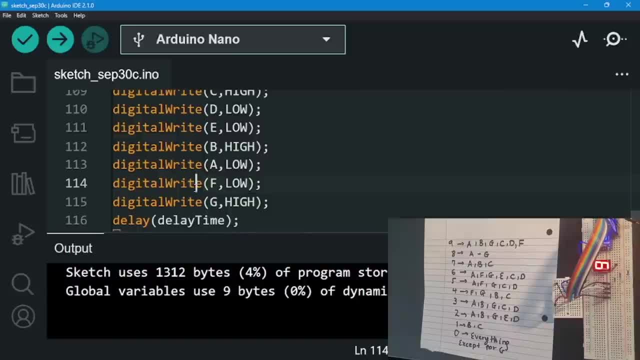 turn that low and f and g, what is left? only zero is left. so let me write down number zero, number zero, and paste that one needs to be turned up for number zero. everything is on, except for what, except for g. so only g is going to be what set to. 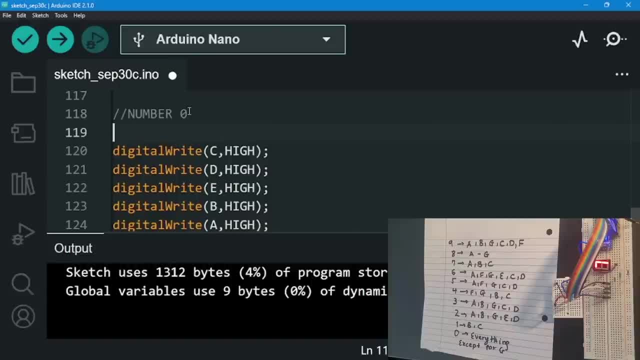 low. one final thing i want to do on number zero is: i want to add: uh, i want to add the decimal point, because we've not been using it. so i'm going to add the decimal points and what i'm going to do is say decimal point and set it to what? to high, okay, so if i'm sending setting this to high, what? 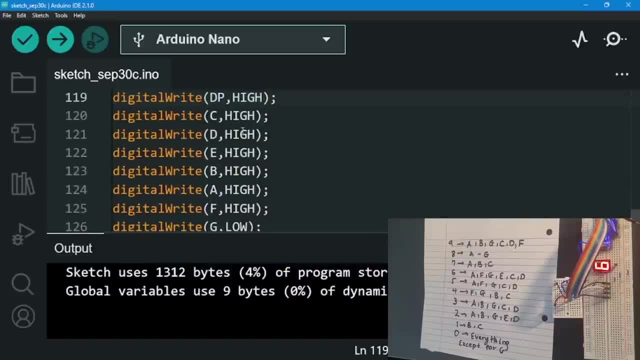 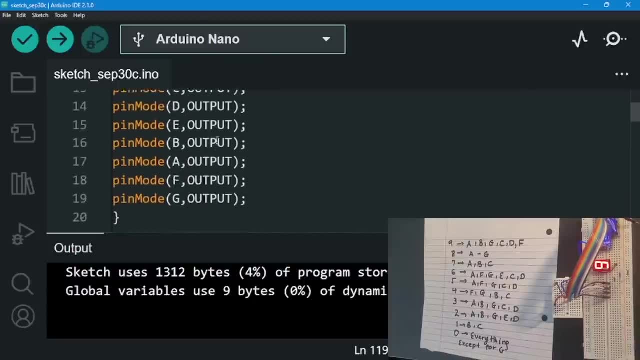 i need to do as soon as this is set to high. after it goes to one round, it's going to kept it high, because i've never mentioned decimal point here. so what do i need to do? i think i wrote it down myself, but what you need to do is what you need: to set it to low. okay, you need to set what the 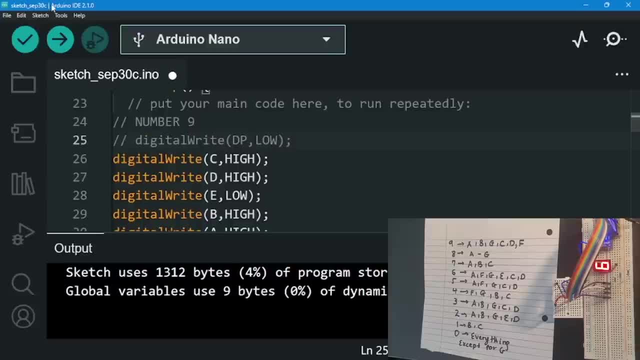 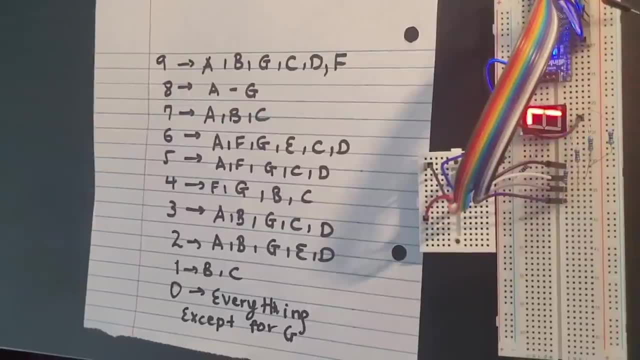 decimal point to low. i just don't don't do that right here and let me just upload it. let's remove it for now. let's see what happens. okay, so nine, eight, seven, six, five, four, three, two, one, zero. okay, the decimal point. you see that, the decimal point after another round, once i set. 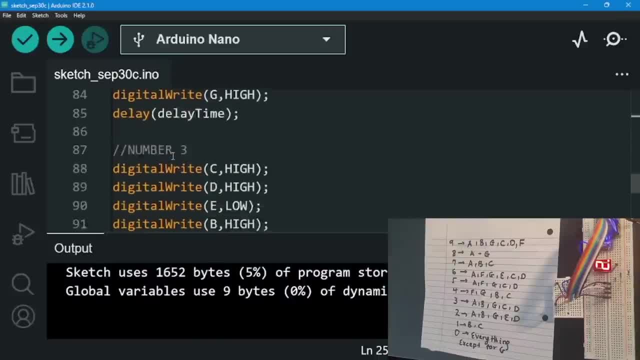 it to high again on number zero when it, when it reaches number zero, i set the decimal point to high, it's gonna what continue on being high as long as i don't write the code to what to keep it on low. so i have to write down the code to keep it on like and not just what neglect it. 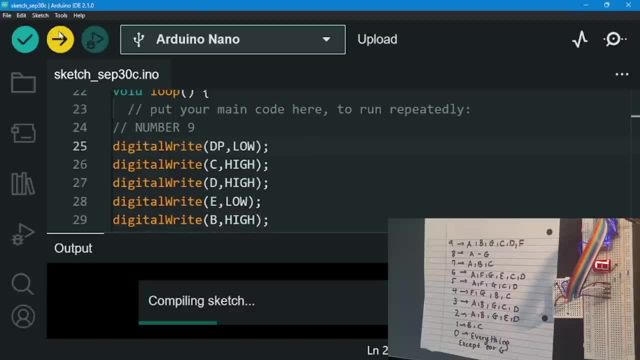 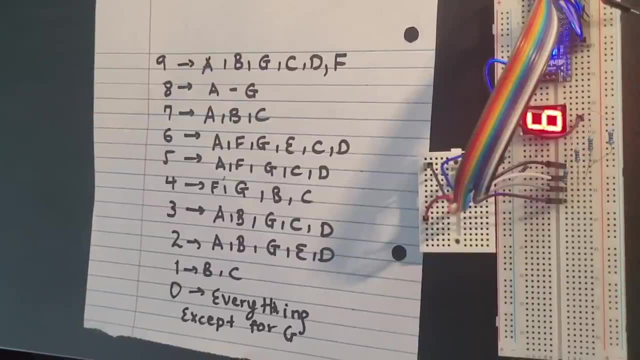 okay, so let me just do that and let's upload it right now. okay, nine, eight, seven, six, five, four, three, two, one, zero, the decimal point, and then the decimal point turns off. there we go now. we created our own timer, okay. so this is as far as we go on the led. 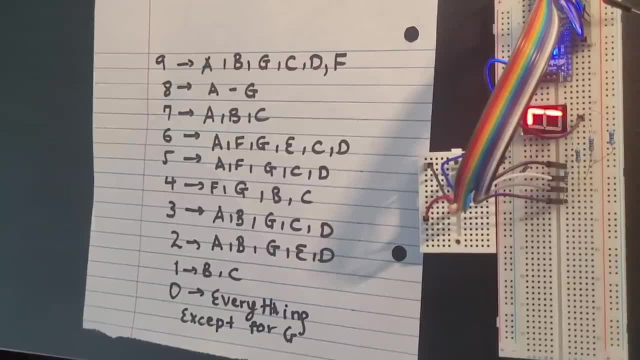 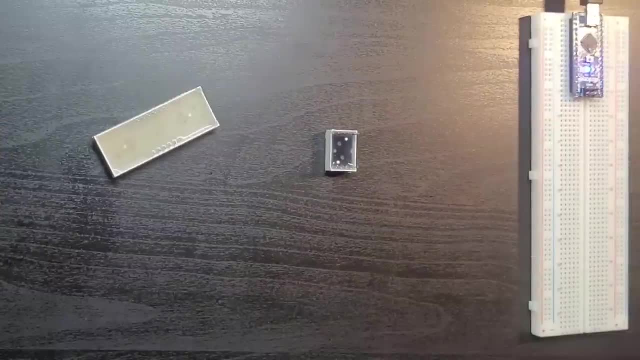 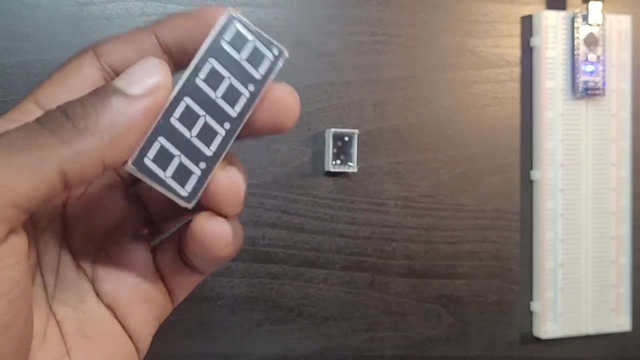 i think we're done with this one, so um, see you in the next section. okay, so in this section we're going to discuss about four digit seven segment led displays. so so far we've worked with a normal seven segment led display, but now we're gonna work with one. 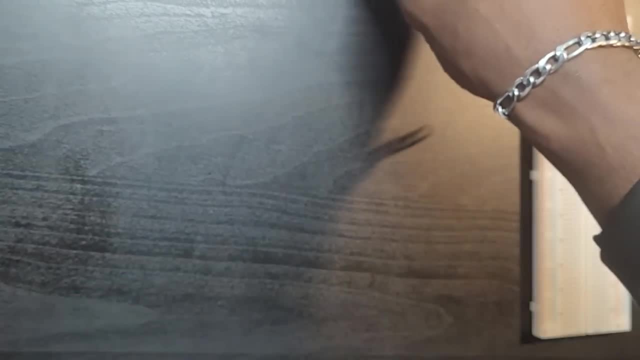 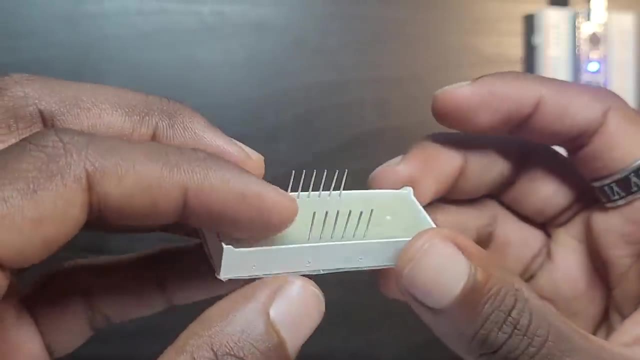 that has a four digits okay. so one thing that you notice right here that is off a bit is when you look at the four digit seven segment led display, is that it only has, as you can see right here has- six pins. right here that's six pins, so totally it has a little bit more. 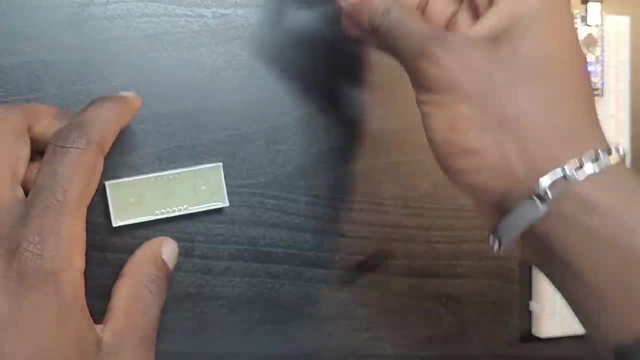 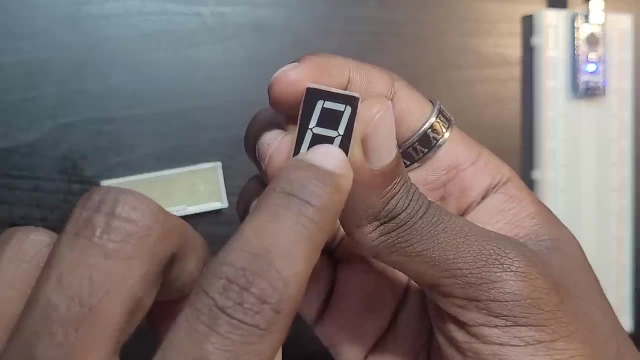 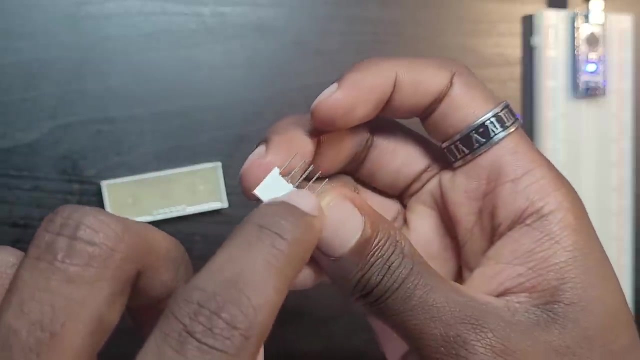 12 pins. okay, when you look at here, when we think of seven segments again, how many pins do we have for each second? right here, we had almost what we have: eight segments, so we have eight, again eight pins for segments, and then we had two pins for the common. as you can see, right here, we have five pins and five. 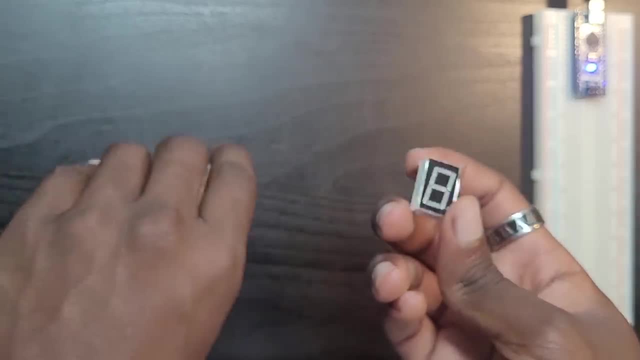 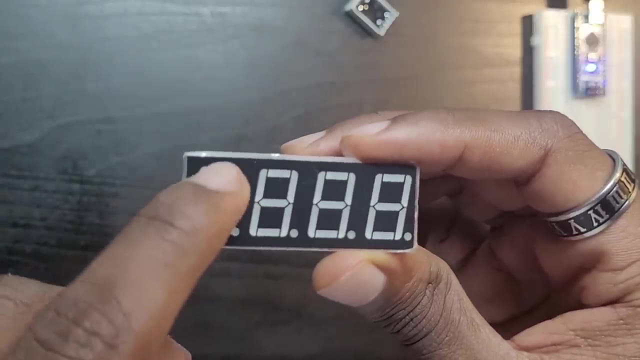 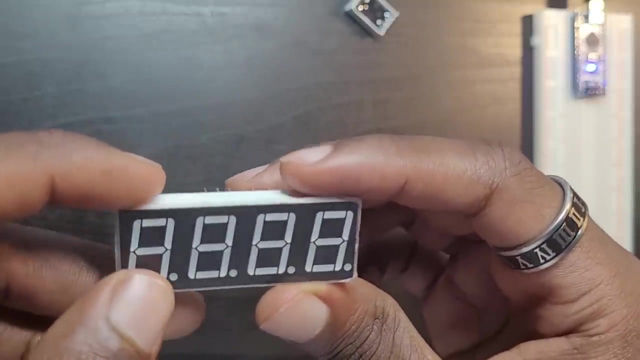 pins. so totally, we have ten pins. so how much pins do we expect? right here, we expected- at least we expected how many pins. we had eight pins, again eight segments here. so we're gonna be expecting how many pins? we're gonna be expecting eight times four, which is going to be 32, and then we expected two. 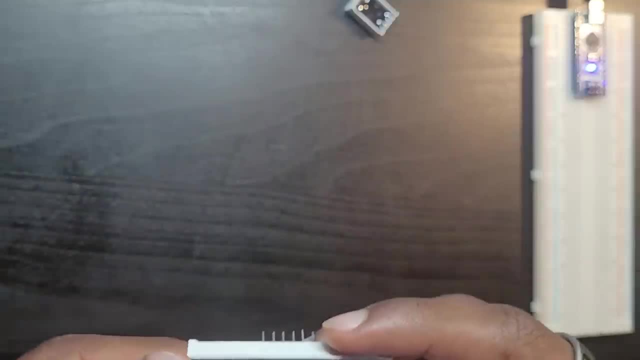 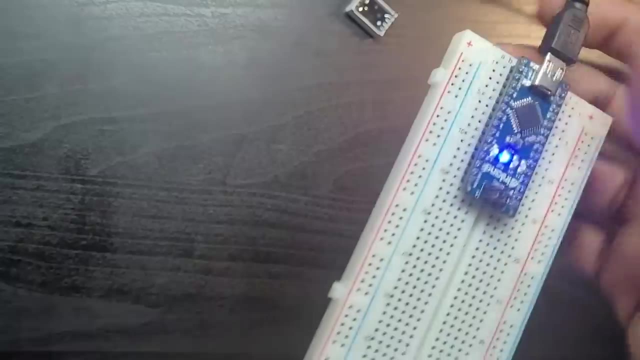 common pins, which is gonna add it up to a total of what? 34, but obviously our Arduino only has how many digital pins. let me just unplug my Arduino so you can see a closed line. if you look at my Arduino Nano right here, it has around 13. 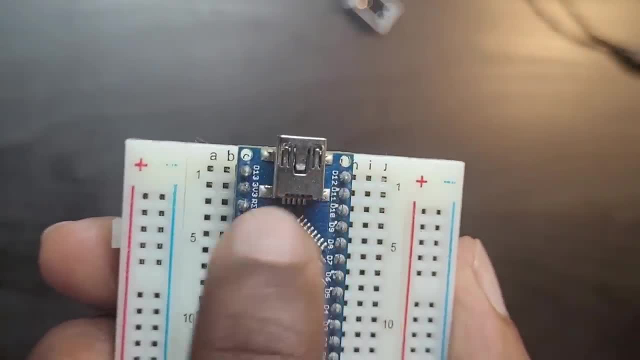 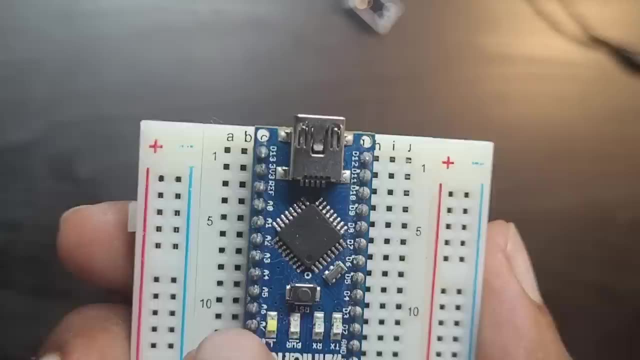 digital pins. it goes to digital pin number 12, right here, and then there's there's still pin number 13 at the very edge. can you see that even let's say we're trying to use our analog pins, we only have how many pins? will we have seven analog pins here? okay, so right here, even. 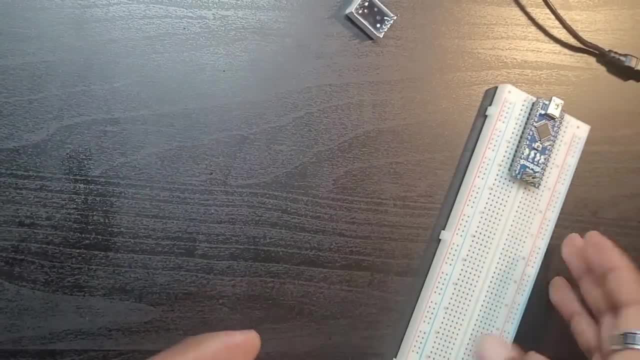 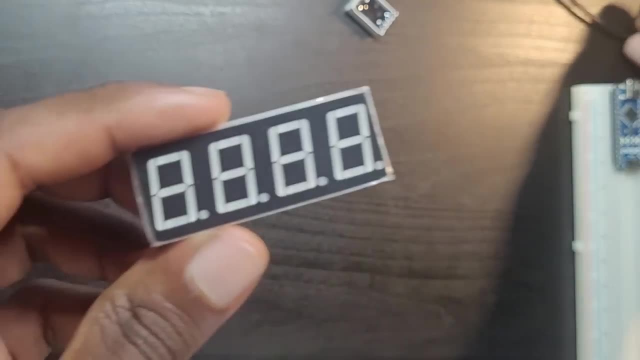 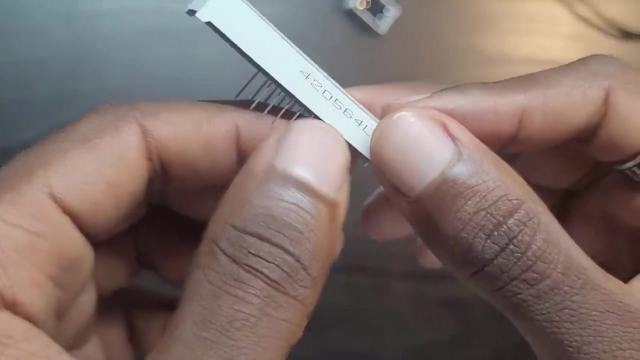 if we add it up, we're not gonna have enough space for 34 pins. so right here they use a very, very simple yet a very genius way of making it, of designing it in such a way that it only needs 12 pins, basically, two more than 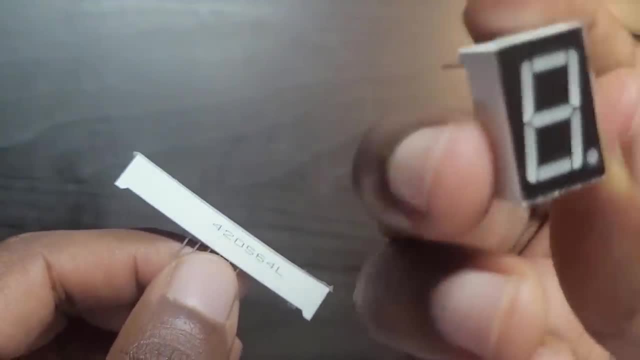 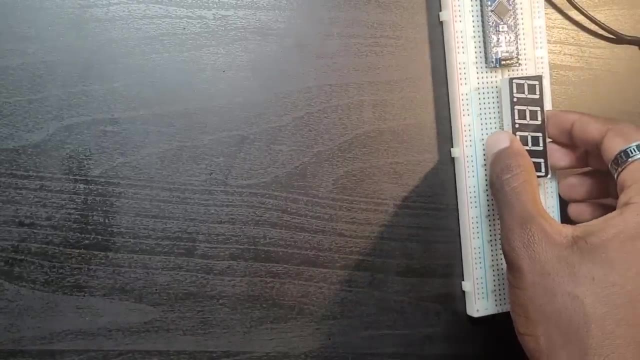 just our normal pins, basically two more than just our normal with seven segment LED display. so let's see how this works. okay, let me just plug my again seven segment LED display. it's very familiar to the LED display we have here. okay, the four digit one is very 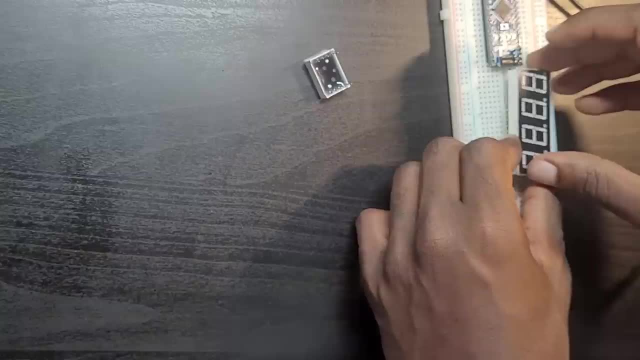 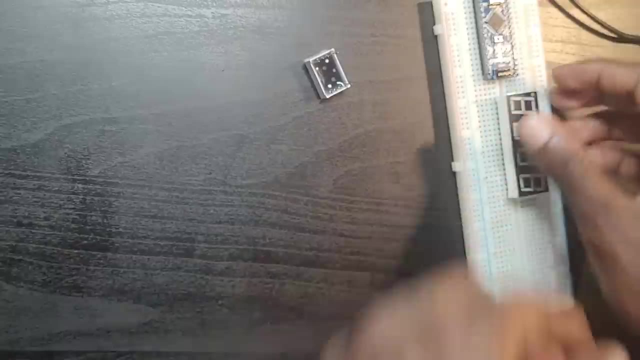 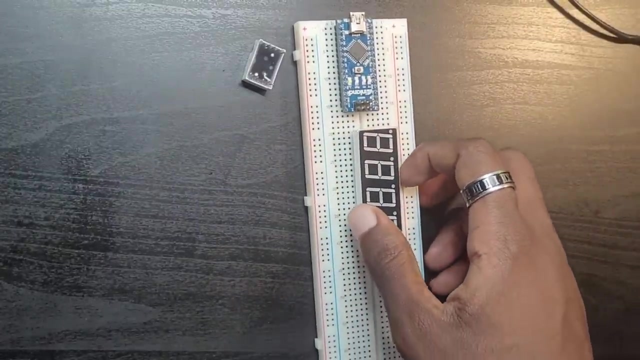 very familiar to this one. let me put it in actually the other side, so it can actually be better. there we go, the focus isn't good. maybe fix up the focus, make it around here. there we go. now it's better. so now the question is: what are these? what are these pins? again, what are these? 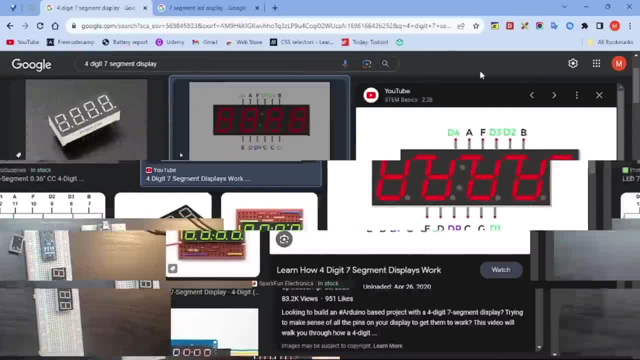 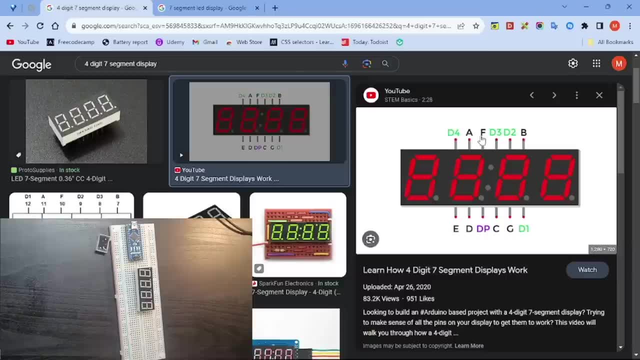 pins. what do they represent? so let me go over to my screen right now so you can see it for yourselves. and when you look right here, there is what there is: D4, A, F, D3, D2, B, E, D, D, P, C, G and D1. so one thing that, again, you're familiar with is are 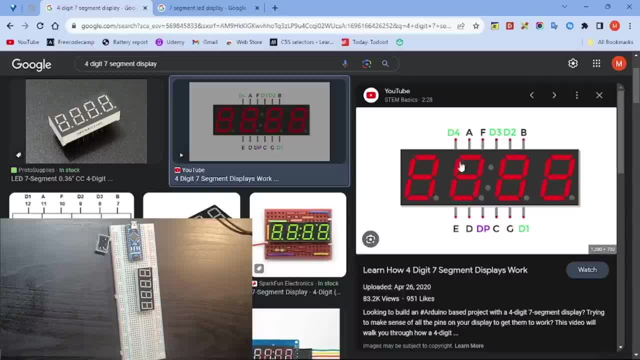 those A to G pins. so you're familiar with the segments A, F, B, E, D, D, P, C and G. we're not familiar with these ones that are marked with the green, the D1, the D2, the D3 and the D4. so D1, D2, D3, D4 basically means is right. I 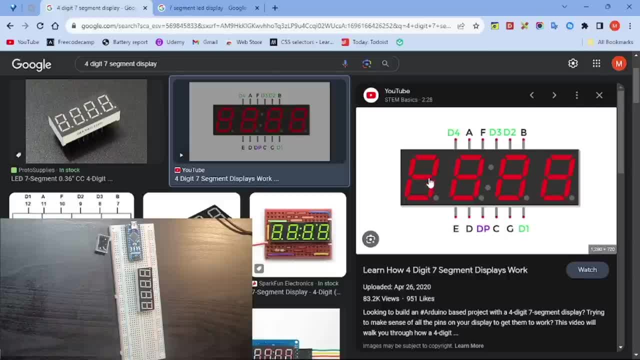 want you to keep this in mind is: D1 represents digit one, D2 represents digit two and, obviously, digit D3 represents digit three and D4 represents digit four. okay, so the question is: what are these these? I want you to think of them. this depends again: these digit pins and what. 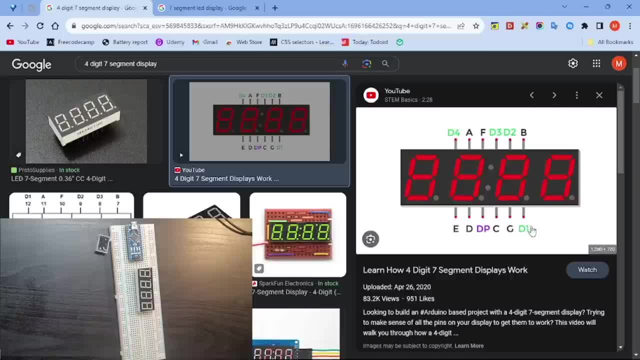 you think of them is as the common pins, okay. I want you to think of them as one, as a com pins, okay. so again, right here, if it's a common anode and common cathode, they exist. here too, we obviously had a common anode, and 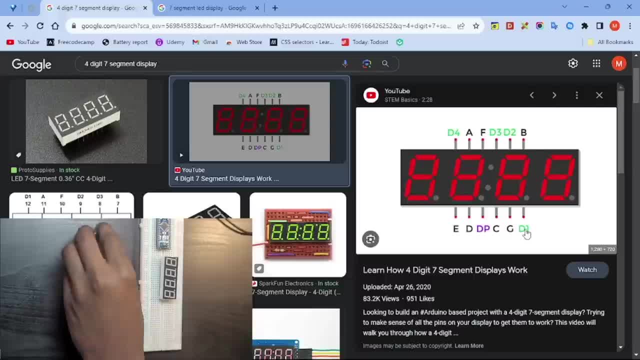 common cathode when it came to the one. when they came to the seven segment LED display. they also exist here too, so there can be a common annode. when it comes to four digit one, it can be common anode or common cathode, okay, so when it 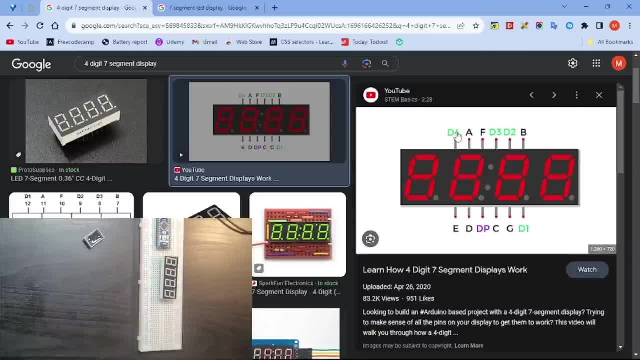 comes to D, again to act as a what, as a common pin. so when you want to turn on something, what basically happens is what. let's say, we want to turn on a on digit four, you want to turn on a on digit four. what do we do is: 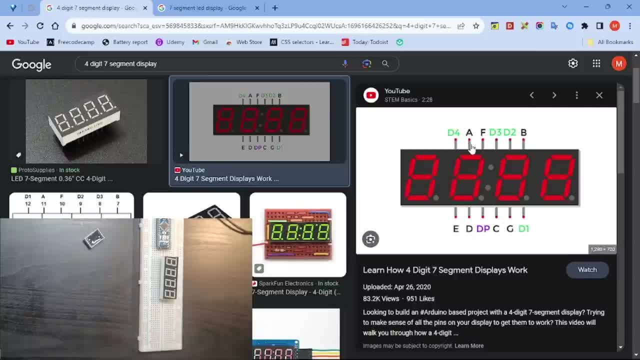 we do what we turn a. for example, let's say i'm using a common cathode. for now i'm using a common cathode. my pin is a common cathode. okay, my uh, four digit led segment display is a common cathode. so i'm going to be using common cathodes as an example. so what should i do? right here? a needs. 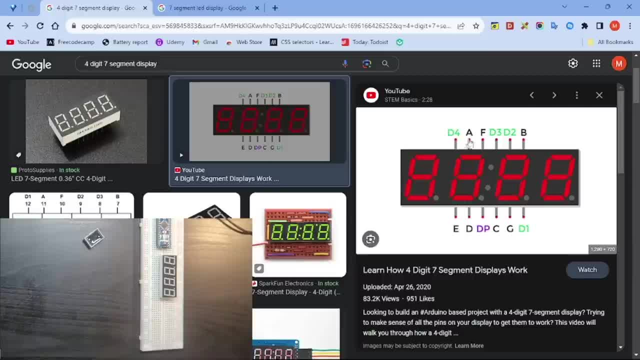 to be turned on to what. a needs to be turned on to high. okay, then the pin that is connected to it's going to be turned to high, and then d4 is going to be what connected to the one. it's going to be connected to low, basically acting as a what, as a ground. basically it's going to act as a five. 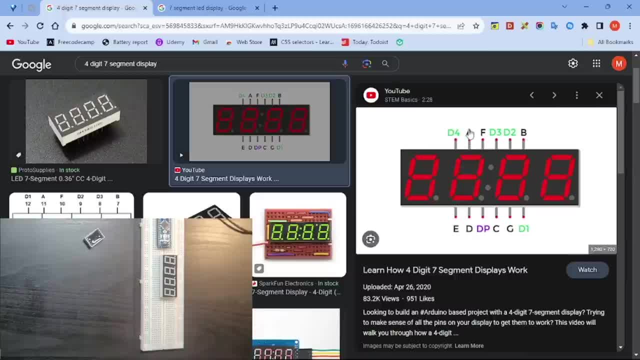 volt, and then there's a resistor right here on the segment. as every time, we did um using the seven segment led display, the one digit seven segment led display, all we did was what. we always connected the resistors to the what to the second. we're still going to carry this. 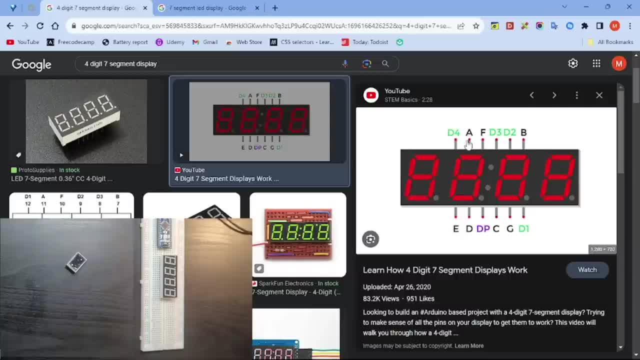 okay, so we're going to be connecting the resistor to the a pin, and then what we're going to do is what we're going to turn on again. we're going to use the d4 as a what, as a gnd, as a gnd common. 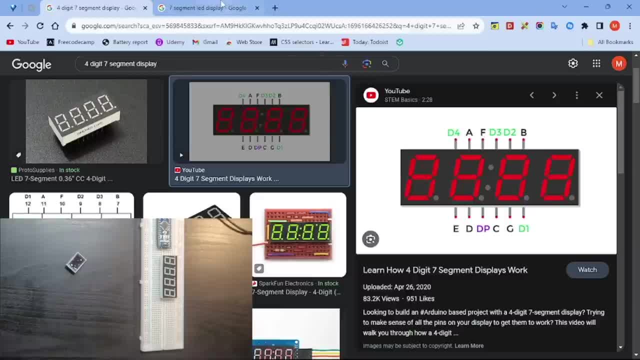 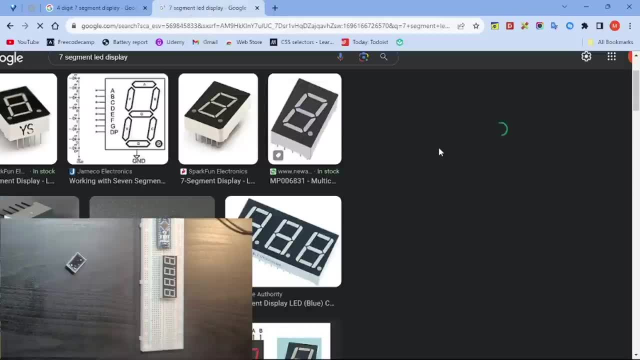 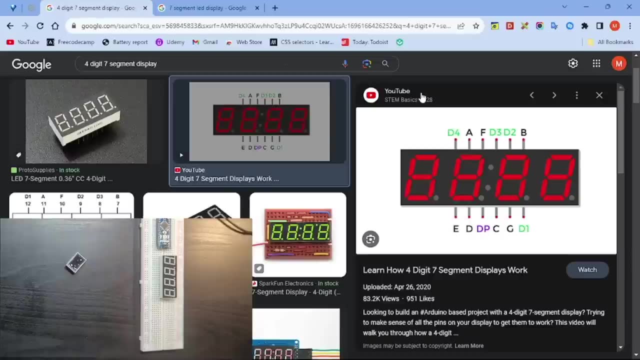 pin and what happens is what we're going to turn on a. where is a supposed to be? let me just google the seven second led display. there's an image before a should be. okay, there we go. the a is right here. the a is right here at the top. so basically we're going to turn on this part. 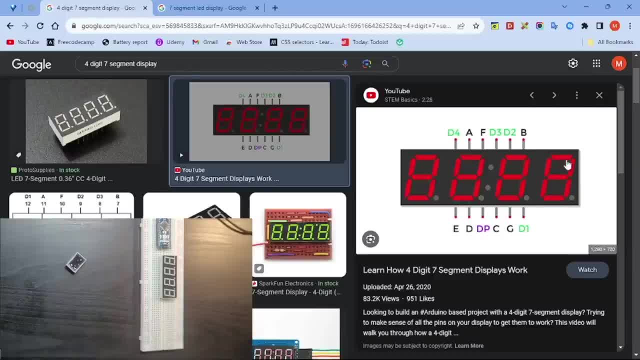 this part. that is what we're going to turn on this segment. it's going to be at the digit four and what it's going to be a okay. so let's try to first things first. let's try to understand. you know how to connect these things, okay, so let me just try to exactly do what i did, right here. 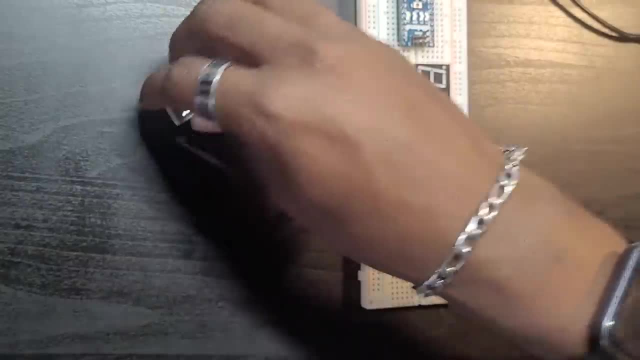 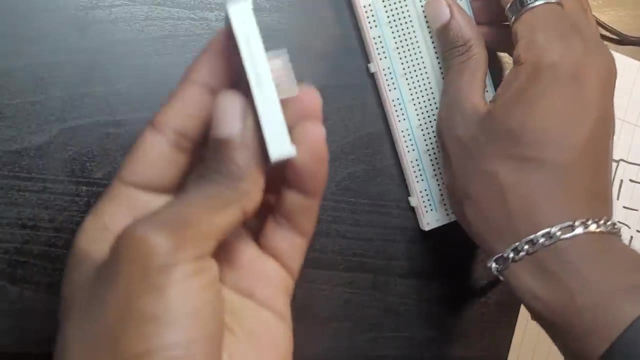 okay, so right here. mine is a bit different again with the number. okay, you're always going to check the number right here. let me just unplug it for now. you're always going to check the number and then search for the data sheet. okay, you're going to search the number right here. you're going to 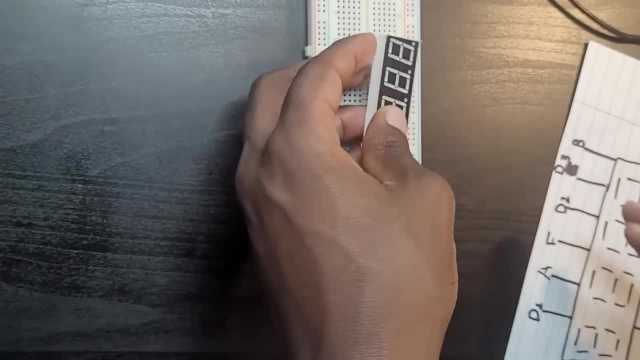 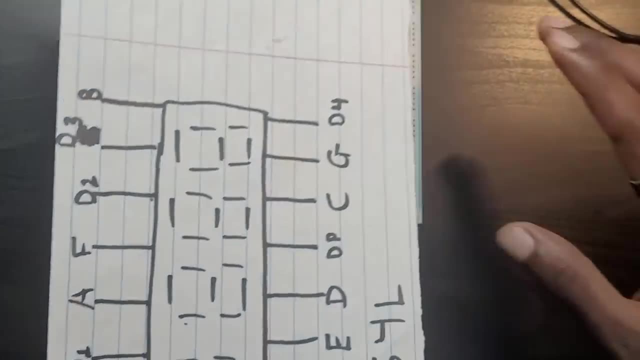 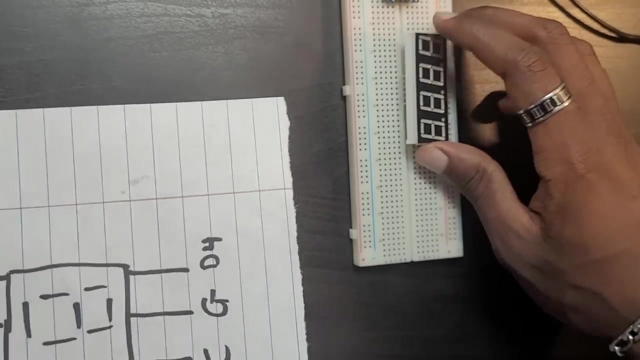 write the number, and then say led matrix, and then what? and then search the data sheet again to just see this layout of how yours is going to be, because it's going to be different from again, from uh, the display to another, so from kit to kit it's going to be different. so again, always keep that in mind. 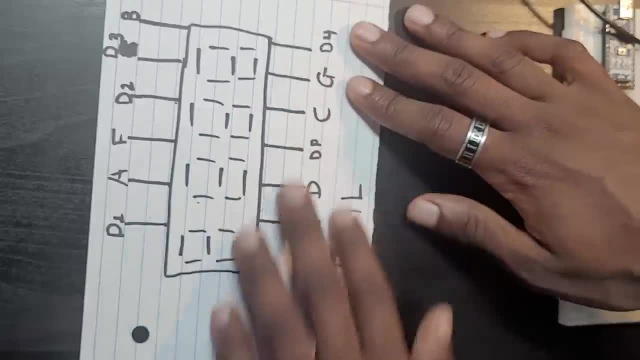 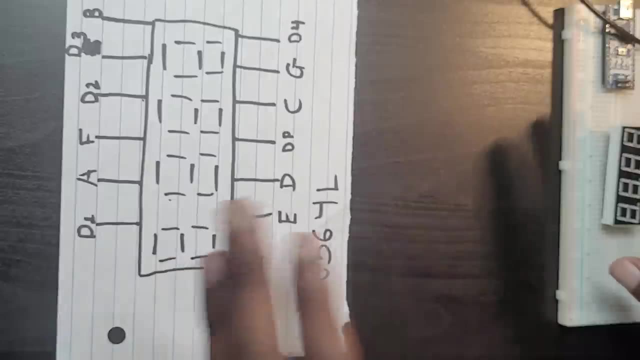 okay. so right here, i already made myself a documentation right here. okay, i'm going to show you guys how to actually make it if you guys do not find the data sheet online. sometimes there might be cases where you don't find the data sheet online- i try to google mine. i put my number right here. i put my number right here and 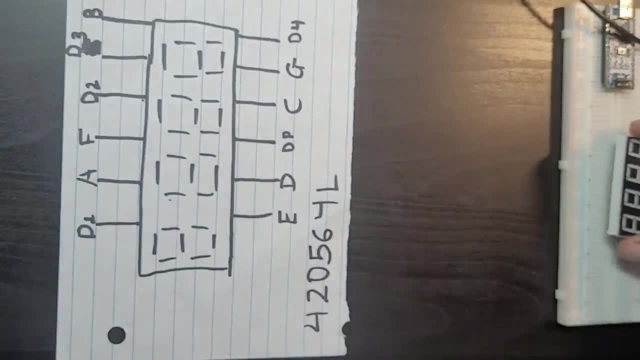 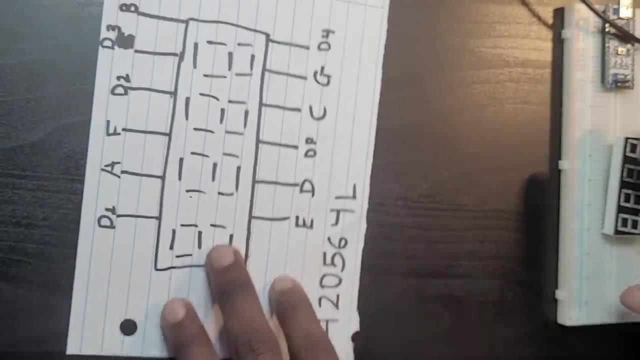 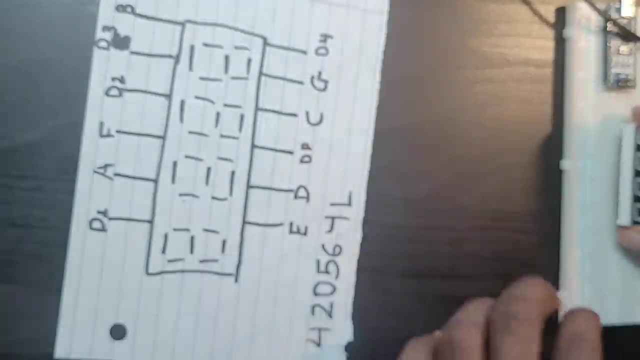 google for it, and then i cannot find it. so what i basically had to do was write a documentation, a data sheet, myself. so i'm going to show you how it's done, but for now let's try to again focus on how- uh, these again four segment led displays- work. okay, so right here, let me just 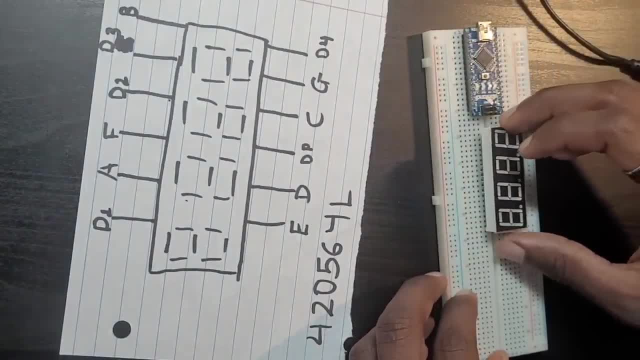 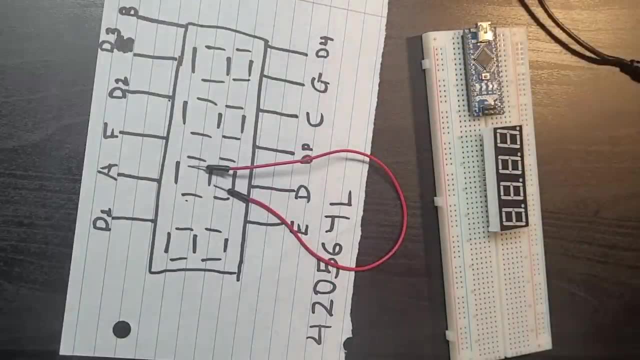 get it as close as possible to the arduino. let's put it right here and bring it to the way i want to, because he's going to copy the data sheet. so let me bring two. bring one resistor here, just bring a resistor. let's bring another wire right. 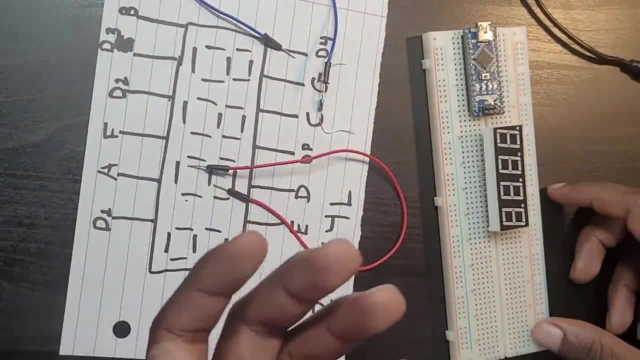 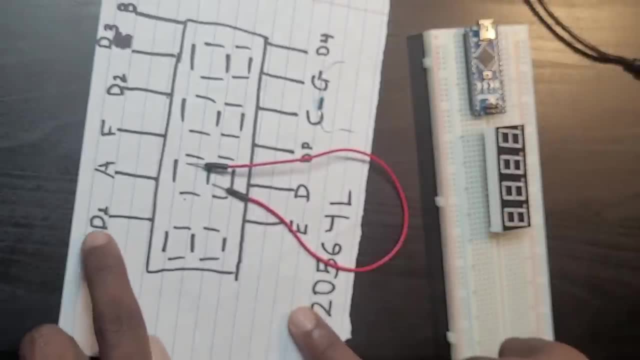 here. mine is a common cap out, so what is the comment pin right here? the common pin for me is what the comment pin is going to be, those e pins. let's say i want to light up digital pin number one here. i want to light a digital pin number one. okay, what do i do? i go to the very edge again. 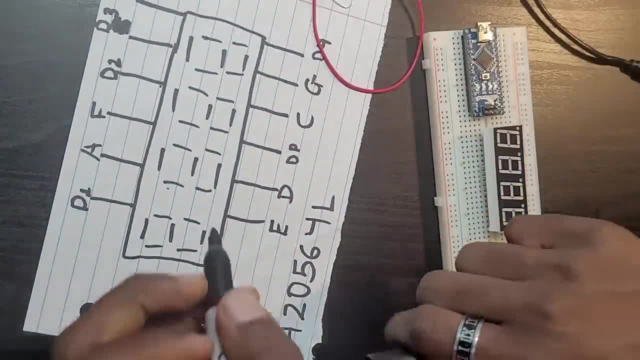 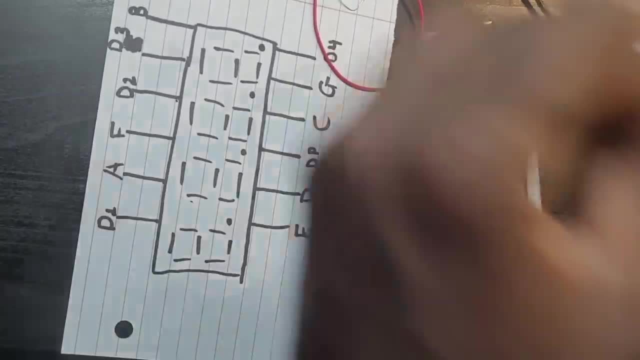 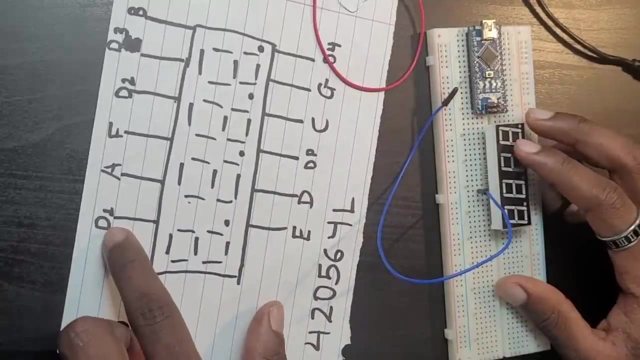 i kind of forgot to put the dot here. let me put 880 here. let me put the dots here. i forgot the decimal point there. we go fix it up right now. okay, so what do i do? i literally put right here. this is going to turn on digital pin one, as you can see, sorry. 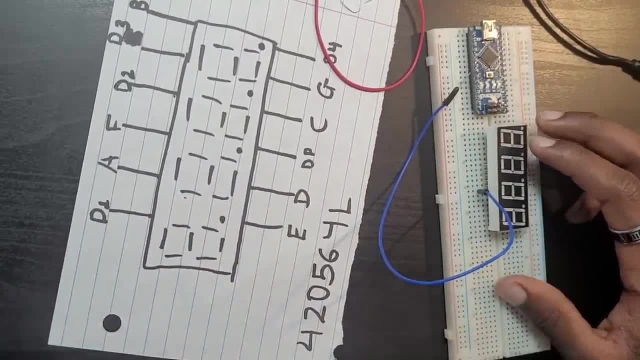 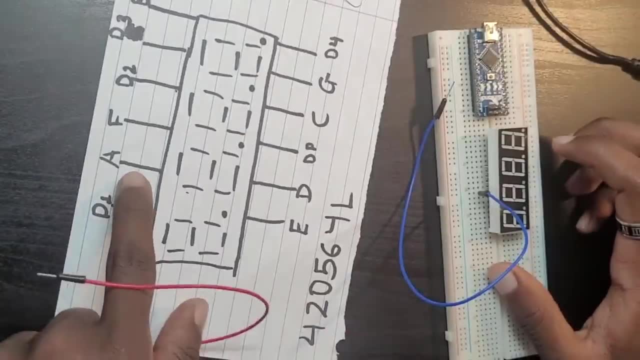 i said, uh, it's going to turn on the digit number one, the first digit, basically, and i want to turn on aim this one. so let me just go right here. but before connecting to a segment, what do i do? i always use my resistor. let me just get my resistor right here, a 1000 ohm resistor. we're. 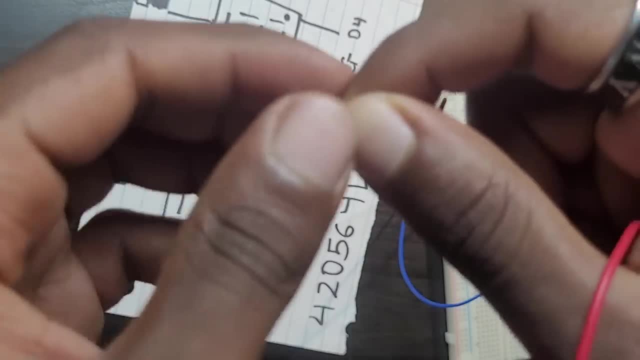 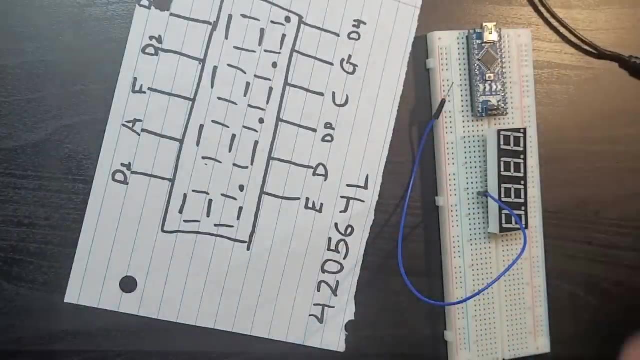 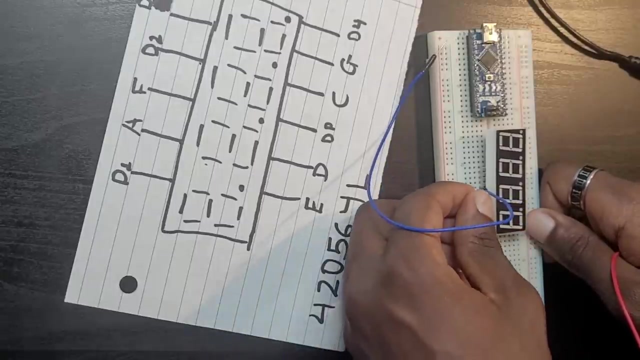 going to be using the same resistance when we were using in uh, in the seven segment, le. in the seventh segment, le displays basically those ones that have one digit. okay, so let me just do that. just try to turn on a. this should be easy. okay, there we go, moved it across. let me just bring. 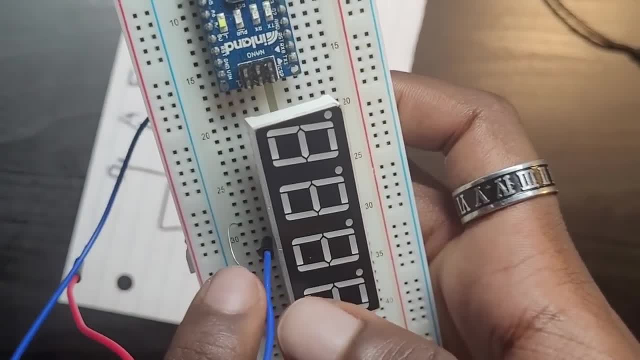 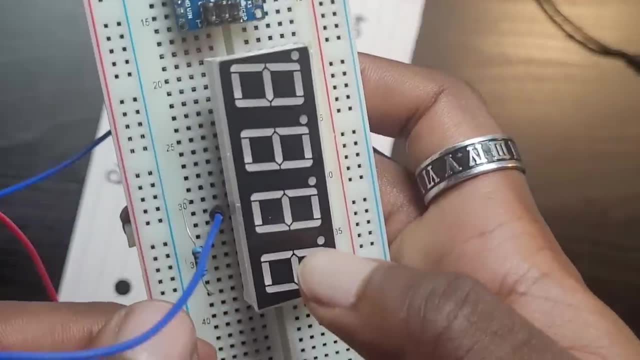 it closer so you can see it again. i connected this one right here. oh, i think i jumped one. oh, i jumped one. actually i'm not correct. there we go. now it should be at a. as you can see, i connected it to a right. everything seems to be working nice now. 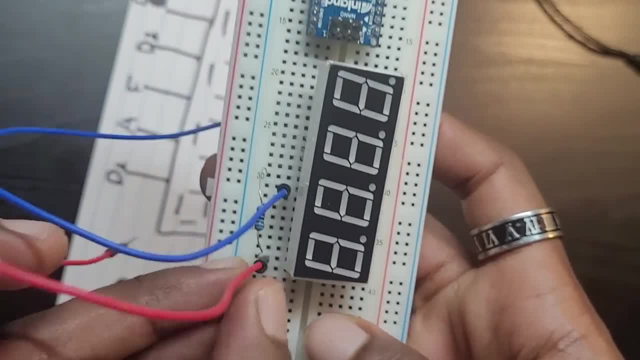 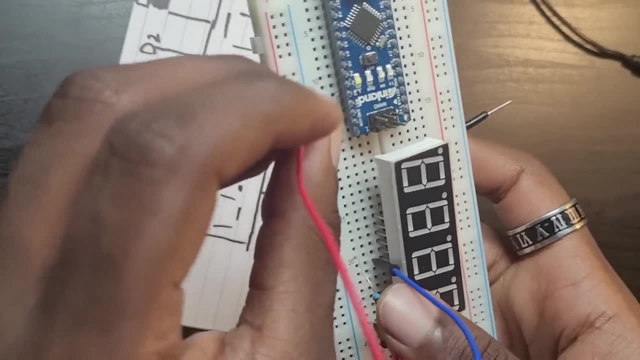 and then i connect this one to the red. so, obviously, what do i connect this one to? i'm going to be connecting this one to what? to the five volt, while i'm going to be connecting my common pin because it's a cathode. again, it's a cathode. this is a common cathode. what am i going? 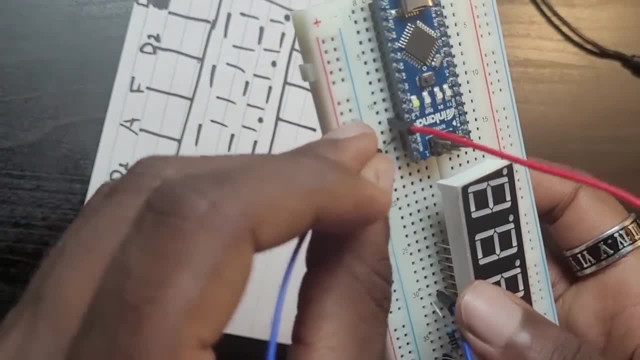 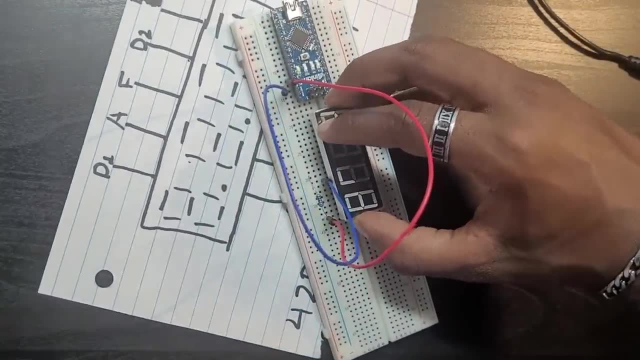 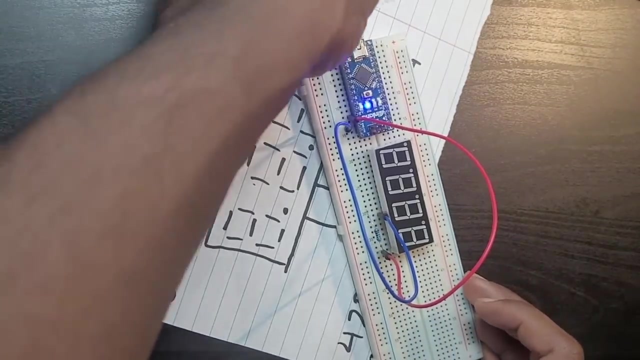 to be connecting it to. i'm going to be connecting it to gnd. let me just do that. okay, it seems to be have been connected. let me just push it in. just need to push it in a bit, and now let's try to light up our arduino with that. let's see what happens here. 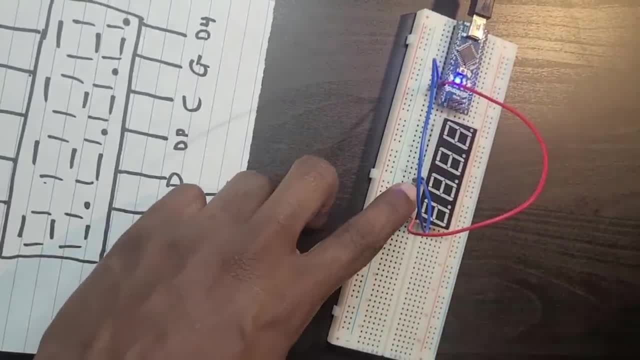 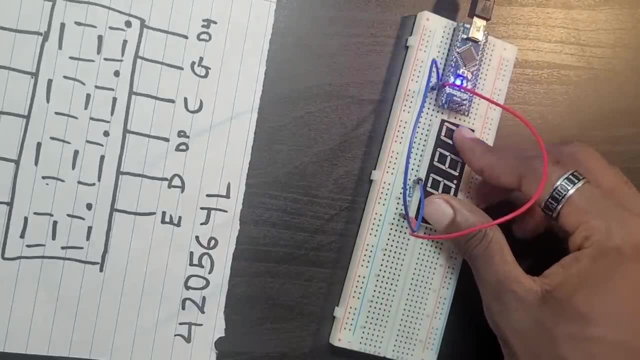 okay, let me just touch my resistors. i'm not sure if the resistor is causing the problem right here. it's not lighting up. let me just try to push it the whole way in. nothing is lighting up right now. we're going through an error. let's just see what happened. 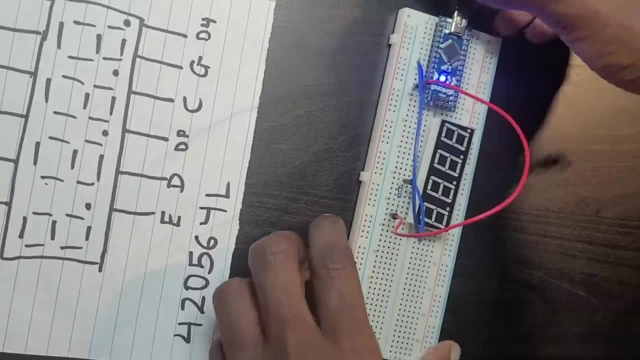 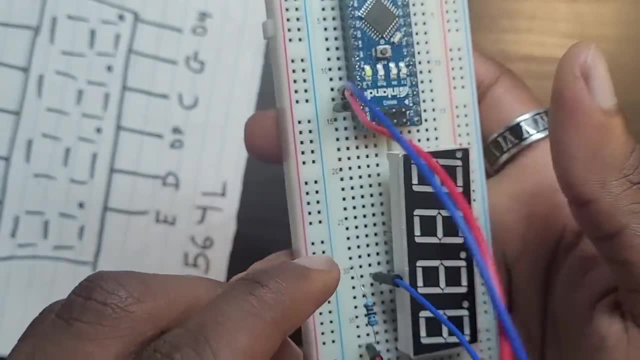 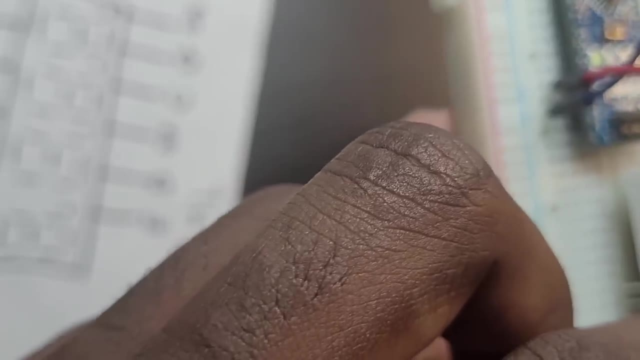 right here again. let me just check my pins. let's unplug my arduino first. let's check our pins. we've been connected in the five volt. all right, i connected the five volt to this one. all right, nice, the gnd. i connected the gnd to this one, which is good. let me just make sure. 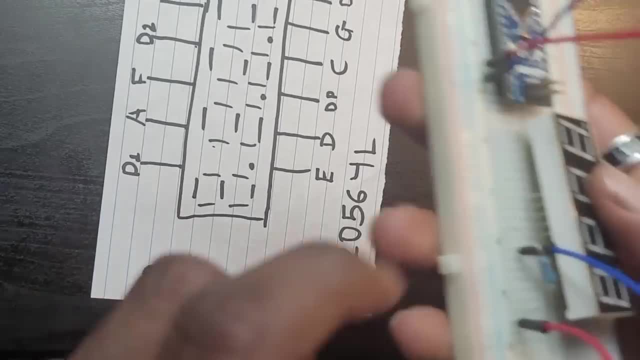 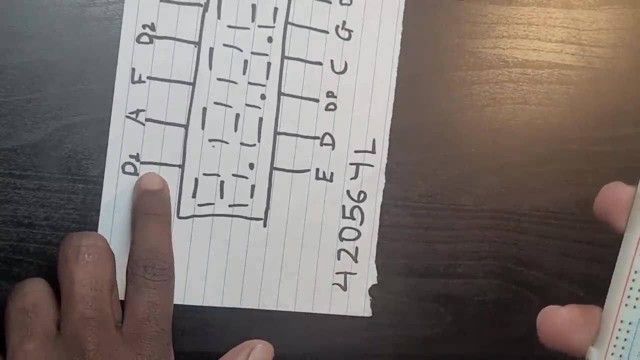 this is what digit one. as you can see right here, this is digit one. let me just check if i connected it to the first pin and i'm going to be connecting it to the second pin and i'm going to be connecting it to the first digit. yes, that makes sense. i connected to what? to a gnd. can you see it? i? 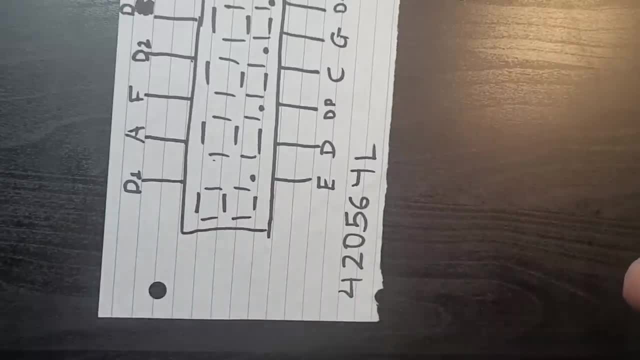 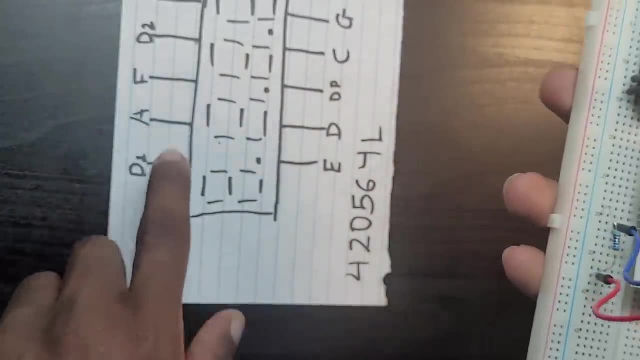 connected it to gnd. and then afterwards, what did i do? and then, okay, connected the resistor right here to an a. connected the resistor right here to what? to an a, the a pin. so, basically, what should have been lighting up this one should be lighting up this segment, should be lighting up this one. 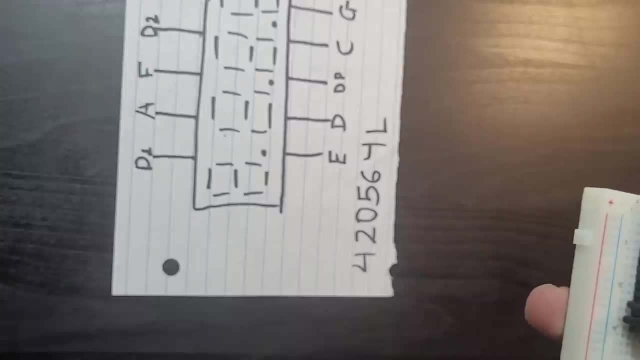 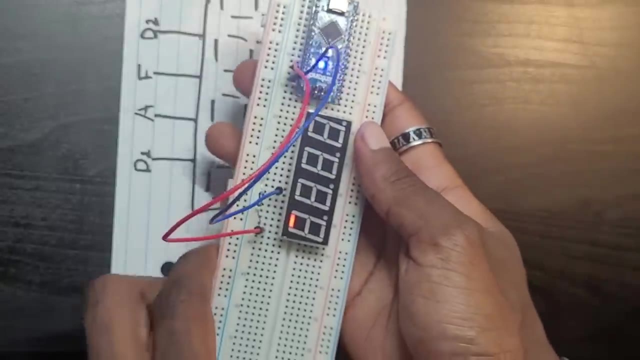 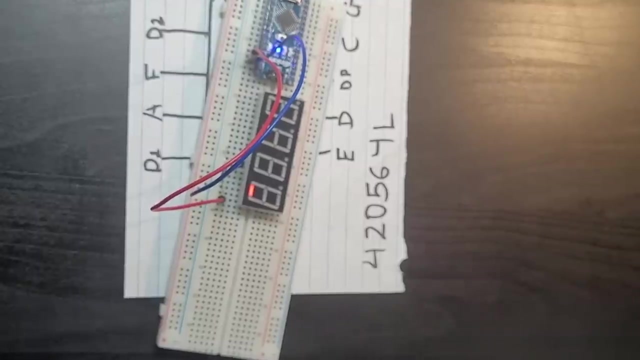 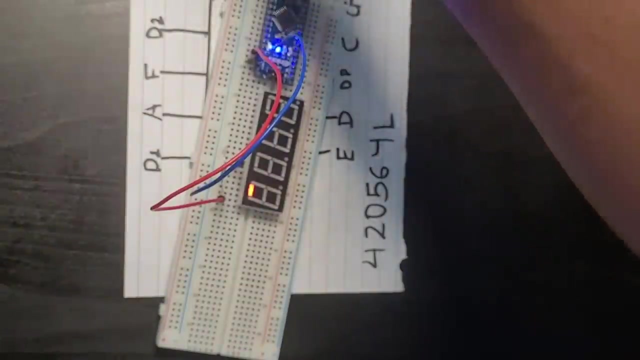 right, here should be lighting up. okay, so everything i think should be working fine. oh, there we go. everything is fine, now it's lighting up. let me just turn off one light so you can see it better. okay, and lower the light a bit. let me give it a different color, right here. 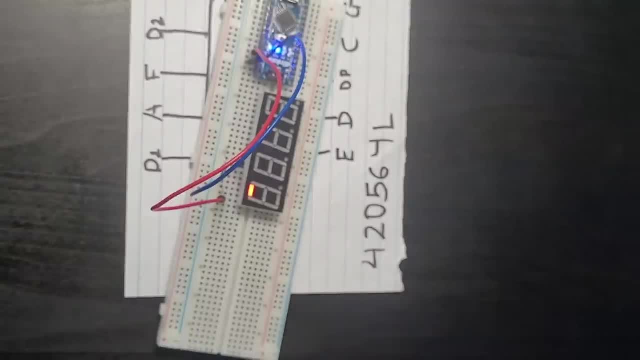 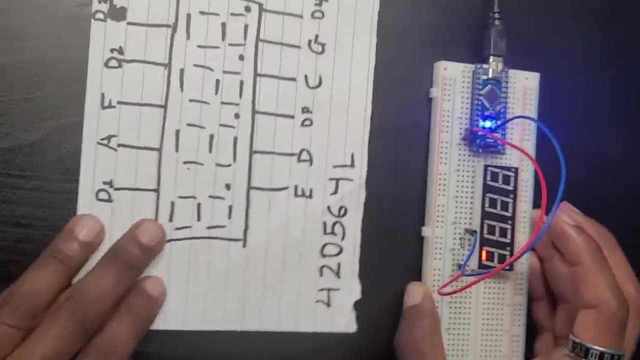 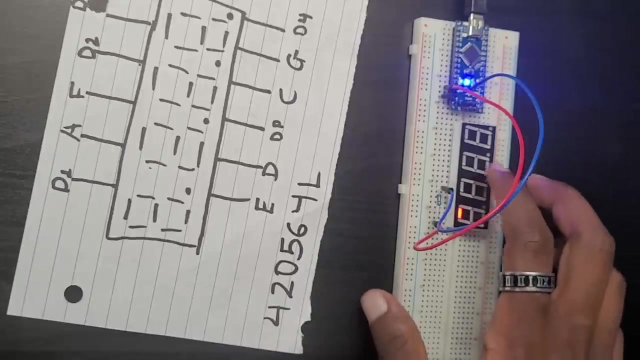 there we go, and now i think you can see it way better. let me try to focus at it. there we go. now it's lighting up, okay, so we just did that, but right now we're going to be connecting the. now the big problem again being here is okay, i turned this one on. let's say i want to turn on. 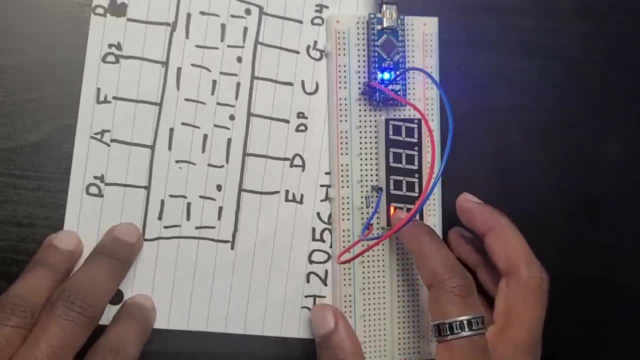 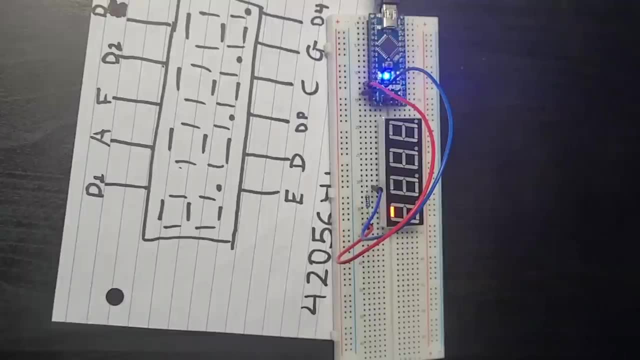 digit number two. i want to work with digit number two now. i just wanted this to be on and i want to work with this number two. okay, there's. number two is what is again, as i'm using, what a common cathode. it's going to be connected to the gnd. all right, where's the digit number two? right here. 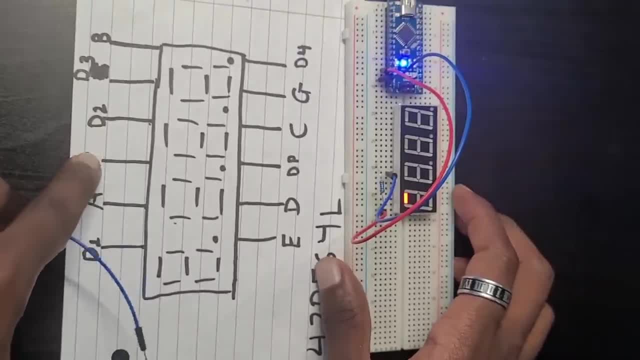 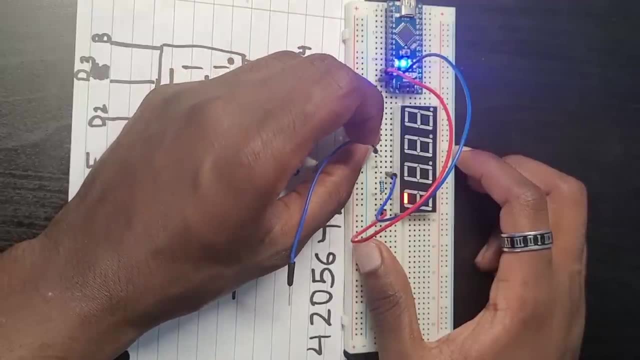 digit number two is after a. i'm gonna have to jump okay in a step and f and then go to d2. let me just do that. so all i need to do is what? go to d2 right here. what else i should do is i'm going to. 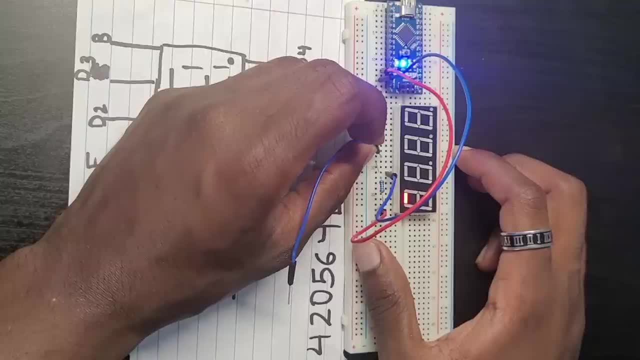 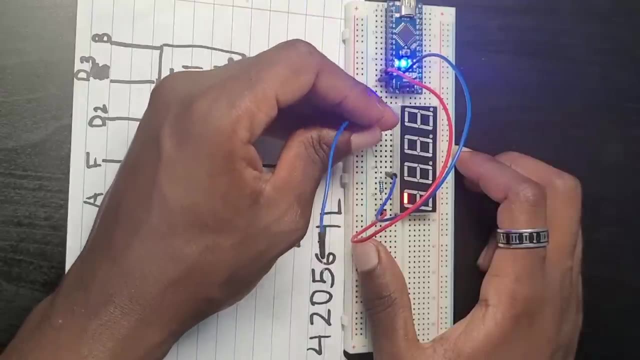 should do is what i should be connecting it to what, to resistor or not? i shouldn't be. why is that? so? i'm working with a what with the common pin when it comes? when it comes to common pins, we don't connect it to resistors, but when it comes to individual segments, we connect it to what we. 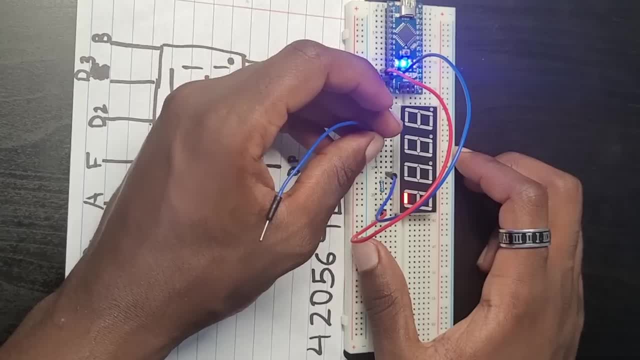 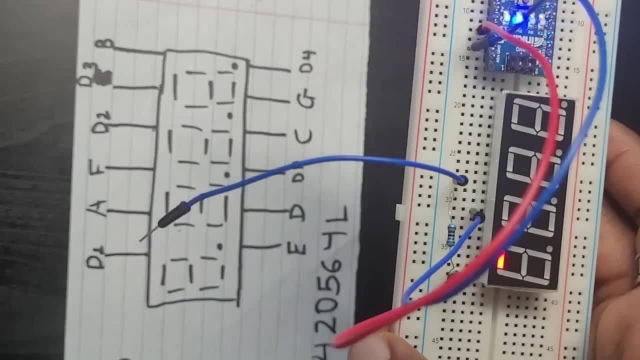 connect it to again resistors. so okay, let me just skip one and go right here. just did that. can you see it? let me just focus here. there we go, skipped it. and now where do i go? i go to the gnd. basically, i'm going to share this. 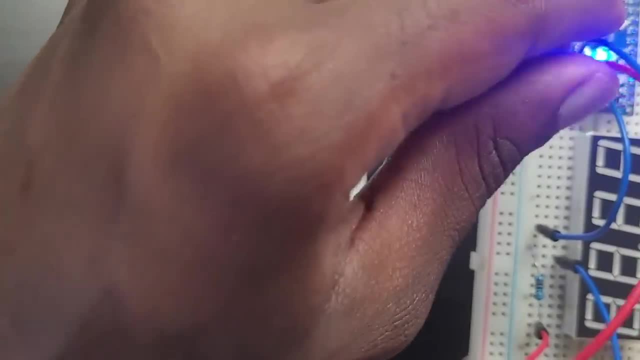 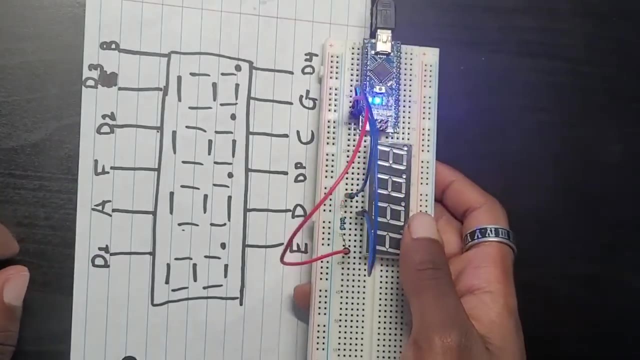 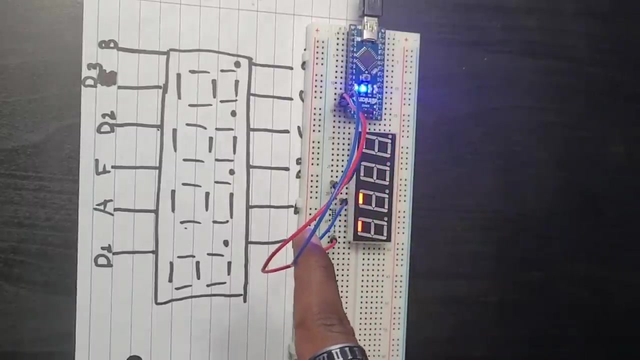 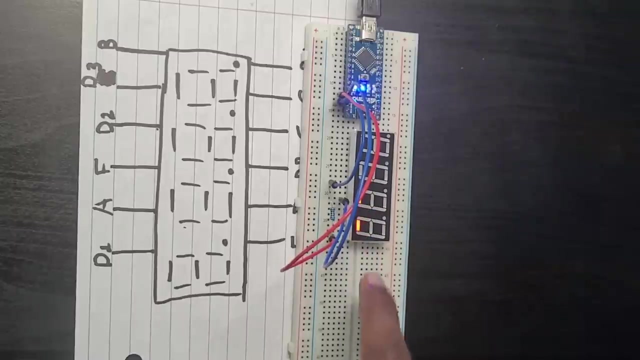 gnd with this. okay, there we go as soon as i do that. can you see that? let's try. there we go, get my resistor. can you see? one thing you notice is okay, seems to be working fine. now let me just try to connect the. you know, i want to turn on f2. i just want to turn on f. okay, there is a problem that's occurring. 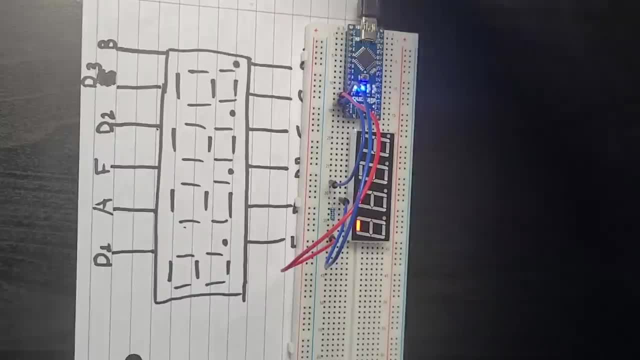 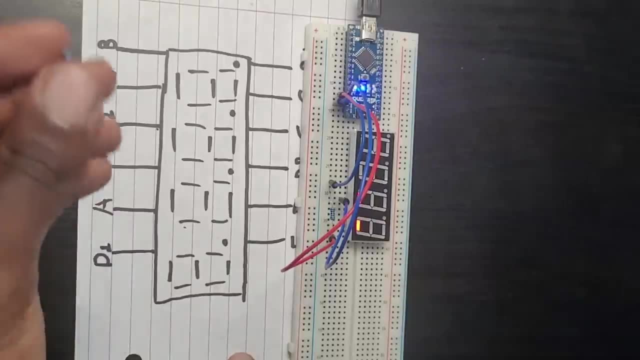 but let's just again go and let's connect it to f right now, and then we're going to talk about the problem of doing this. let me just connect it to an f right now. okay, how do i connect it to an f? i'm going to need again a resistor right now because i'm lighting up one, an individual segment. 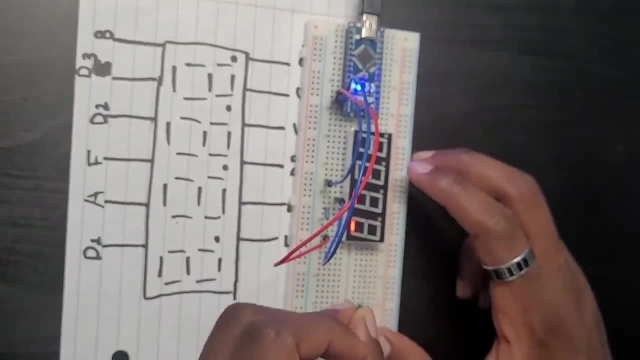 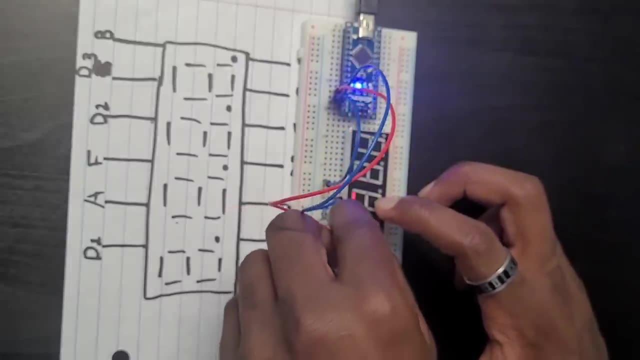 all right. so i'm going to what i'm going to need to connect it to an f. so where is it? it's around the middle. i have to go between these two. yep, it's just going to be a bit of a hard one. it's going to. 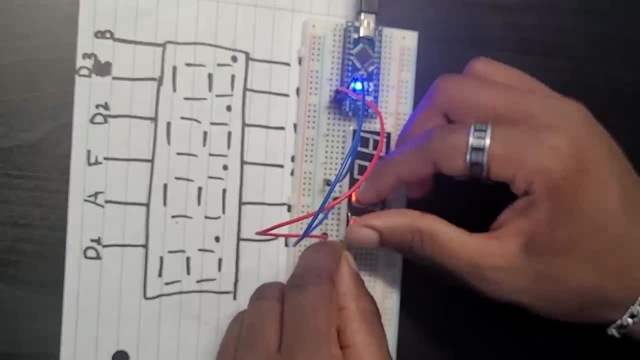 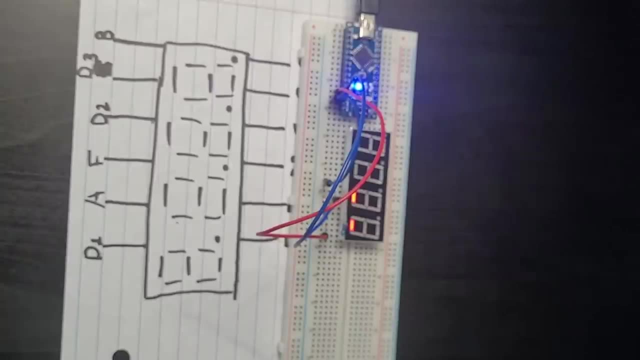 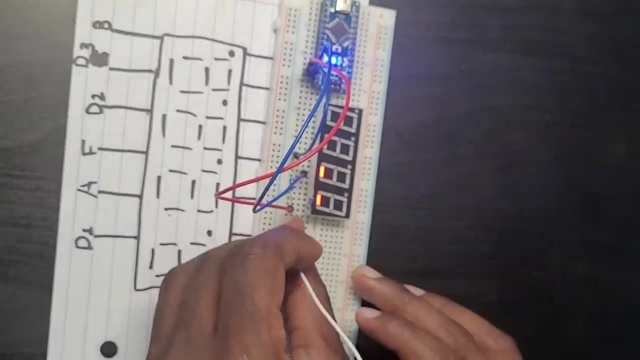 be a bit of a hardship to do actually. all right, there we go, connected it to an f and then i'm going to need a wire. i'm going to do long wire. actually this time i'm going to get the white wire. it's very long. there we go. what am i going to be? connecting it to? the five volt because i'm using a common 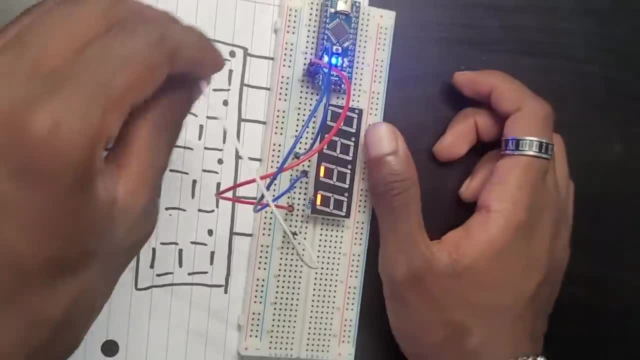 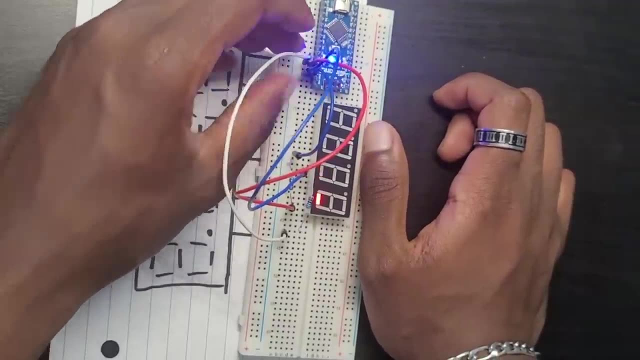 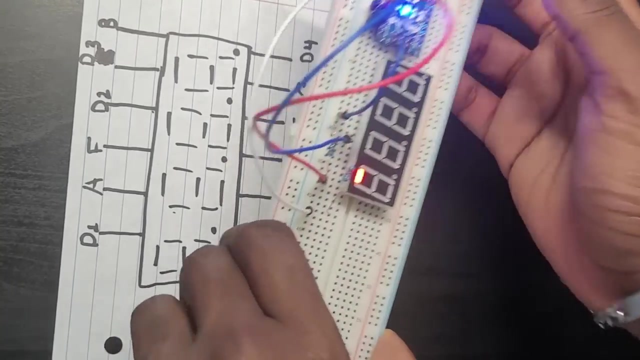 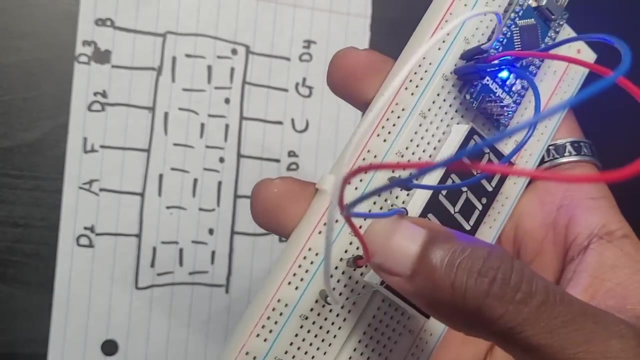 cathode. again, the individual segments will be connected to what? they'll be connected to the five volt. let me just do that. it should be connected to the five volt, which the resistance. let me just check both resistors. all right, there we go. just touch the resistance right here. can you see a problem occurring? it's not consistent, as you can. 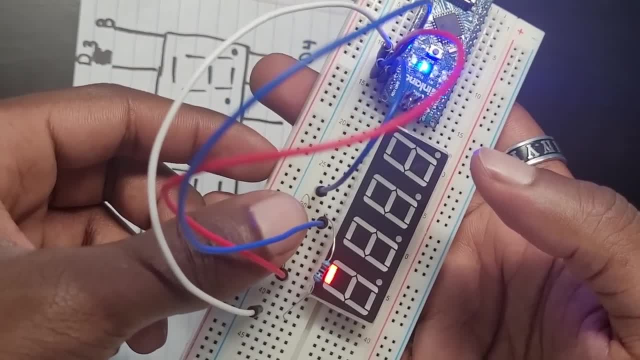 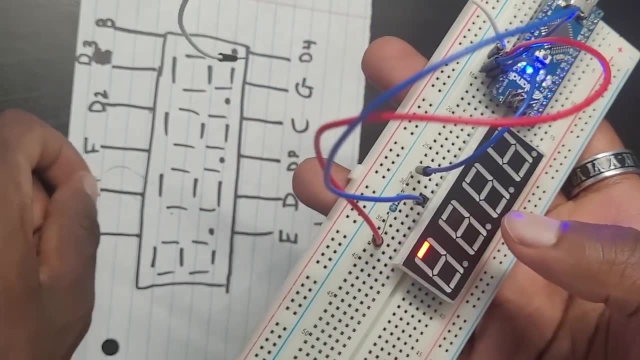 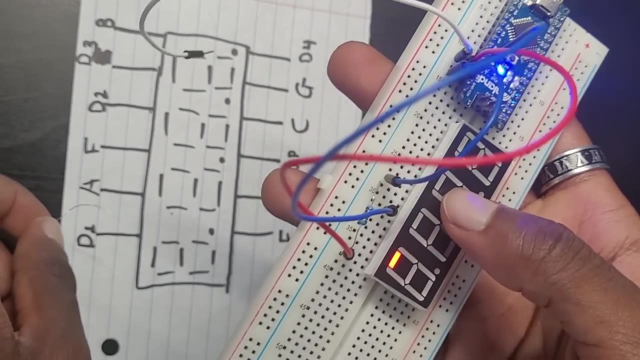 see, it's not really consistent. what is the problem here? the first problem is: okay, the first problem being we just take off this one. just take it off for now, so you can see it. the first problem was: there is not what, there's not enough power to turn off, to turn on all these displays. okay, that is the first problem, okay. so, as i said, 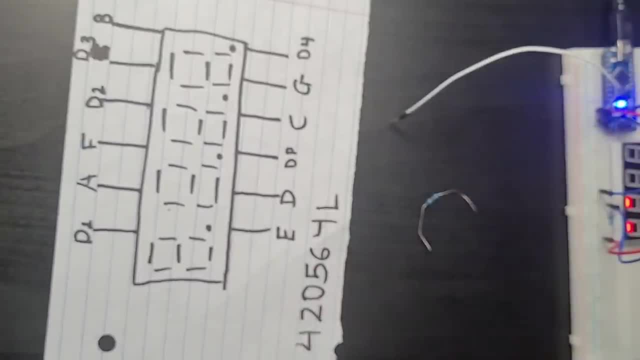 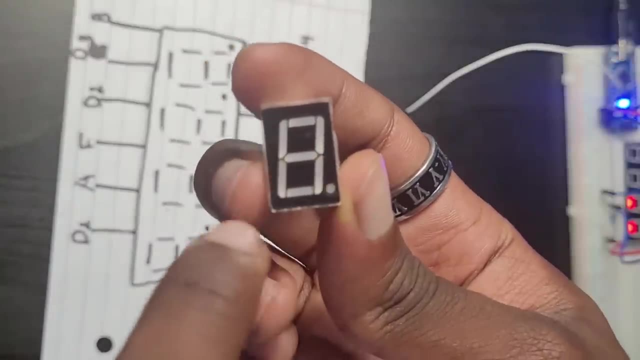 again. these again when we're when we're putting our resistors. they were intended to what they were intended to for what? for one segment led displays. they were intended for one segment, what led displays? so basically, we turned on its maximum. we turned on eight segments here, remember. 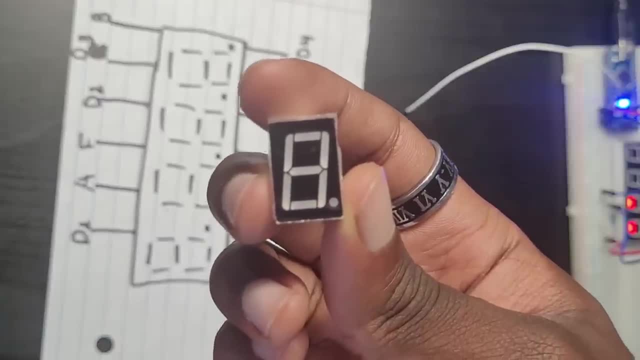 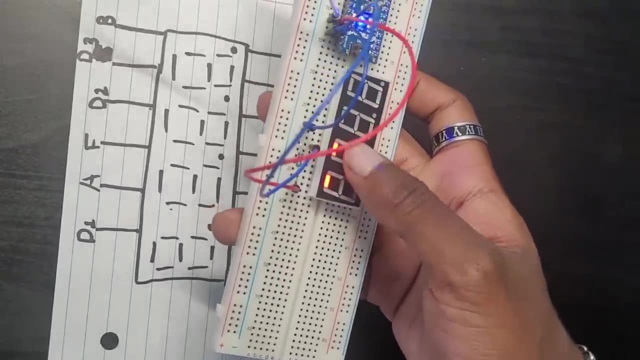 maximum. we turned on eight segments. just think of them lighting up what eight leds here. all right now, we have how many segments we have around eight right here. eight, eight, eight. basically, we have 32 segments. how are we going to light up 32 segments? because it's going to require. 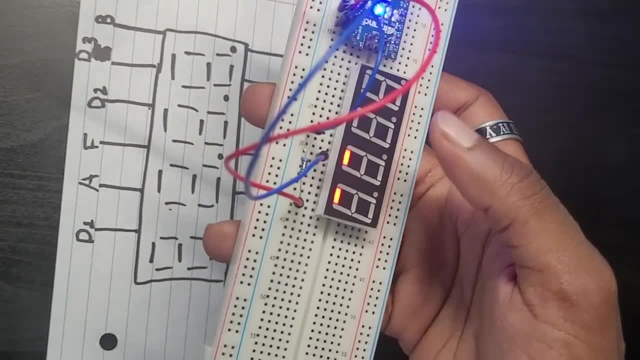 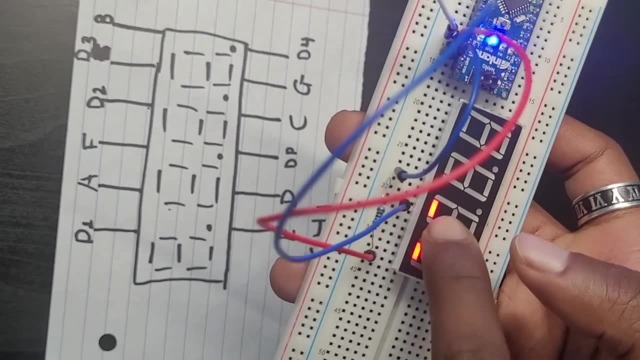 a lot of power. it's going to require more voltage than five volt. okay, so one thing we could have seen right here is when i put the f pin right here, when i connected, try to connect the f pin, everything, what everything blacked out. what happened basically was it did not have enough. 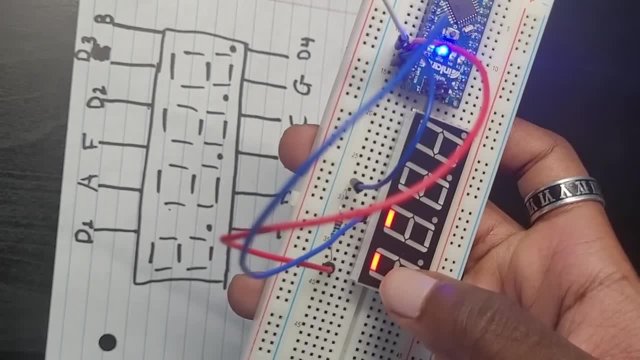 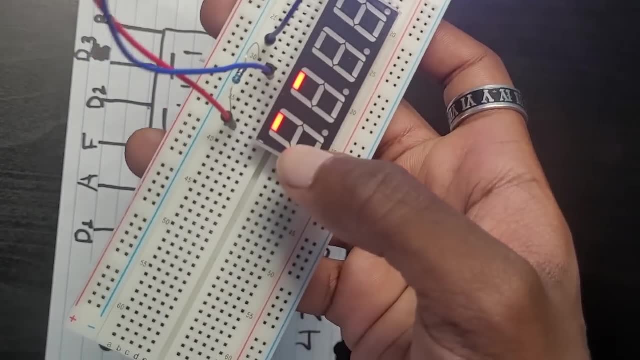 power to light up all of them. okay, did not have enough power to light up what all of these segments were, and so now we're going to try to connect the f pin to the led display. and again, okay, that's one thing i just want you to keep in mind: they had no enough power to what to. 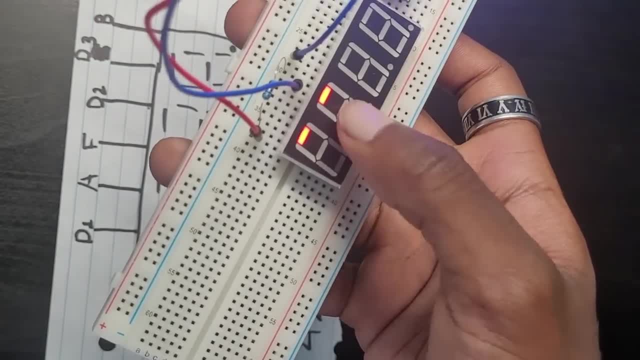 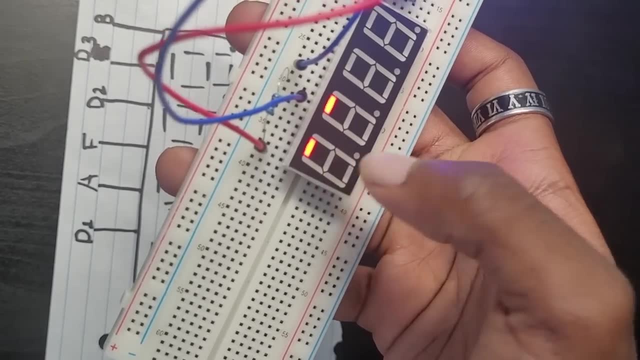 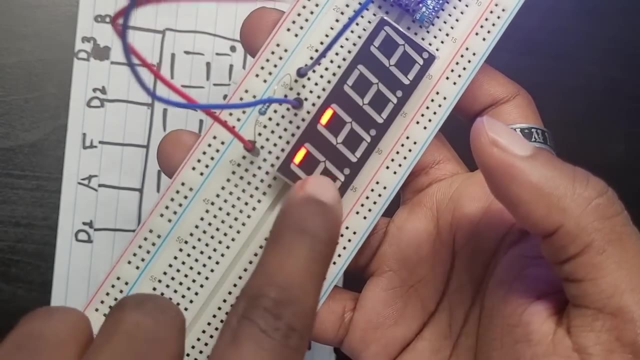 light up again two, again two different digits. okay, so right now. another problem is it starts copying the same thing. can you see it? if i just put right here a right here, it's going to light up both. let's say i want to turn on one. let's say i want to turn on, i want to represent that one, two. 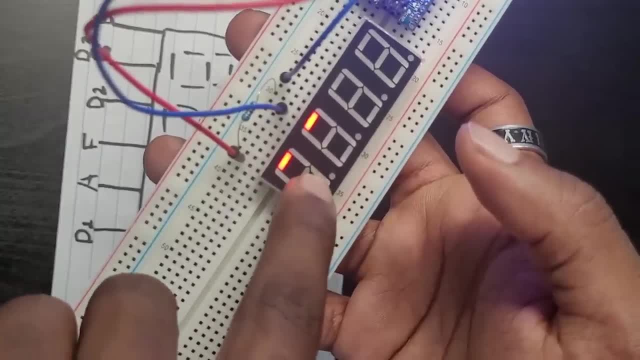 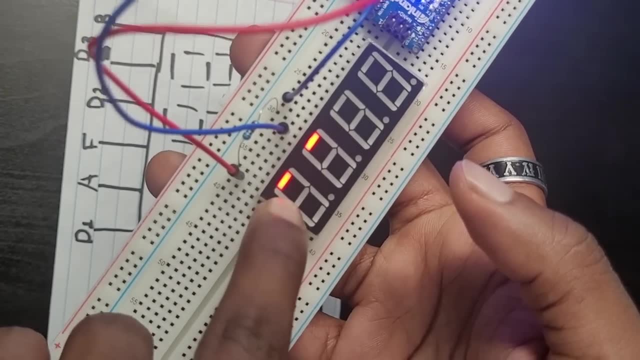 the problem here is what. okay, i need to turn on this and this for number one and i'm going to turn on another type of what, another type of segment for number two. but right here, what happens is what? it copies the same segment. so when i light it up in this manner, what happens is what. 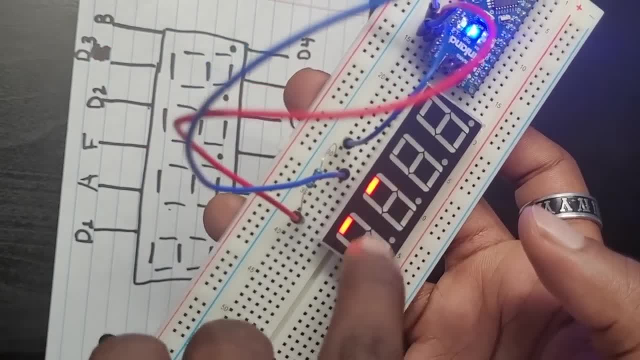 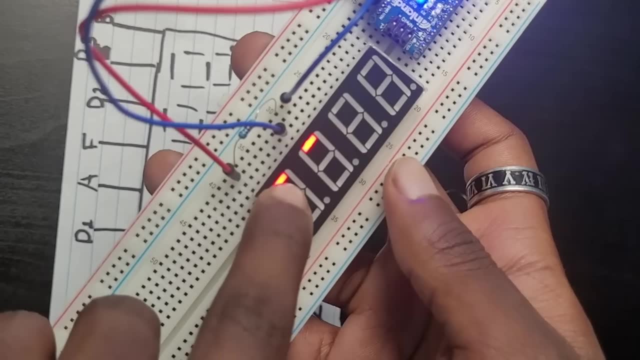 it lights up what it copies: the same thing. it copies the same thing. so it's going to be what it's going to be very, very horrible. you don't want it to be exactly the same. as i said again, let's say i want to turn on one right here, and once i want to turn on two, they're going to be. 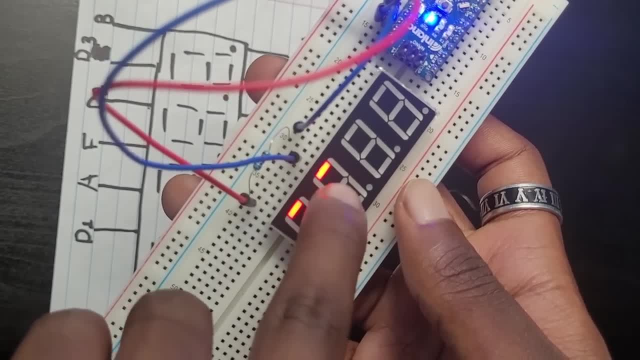 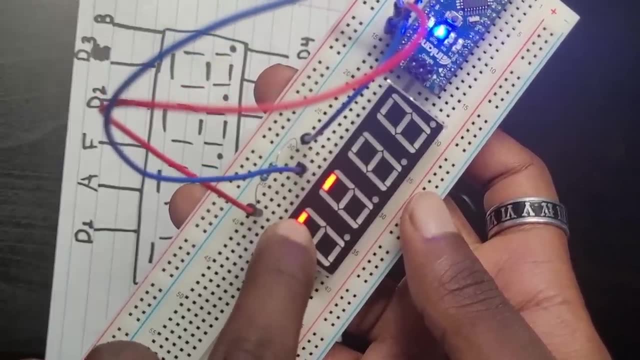 a problem right here. let's say, i turn on two, okay, i'm just going to add up these segments right here, just fine. but when i want to turn on one, what happens is what? i have to turn off this one. okay, i've turned off this one. so, basically, what happens is what? if i turn off this one, it's going to turn off from. 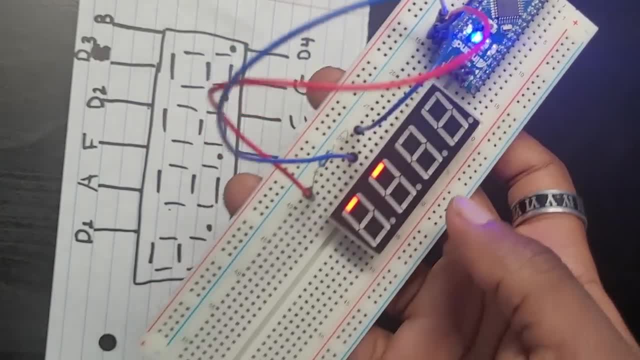 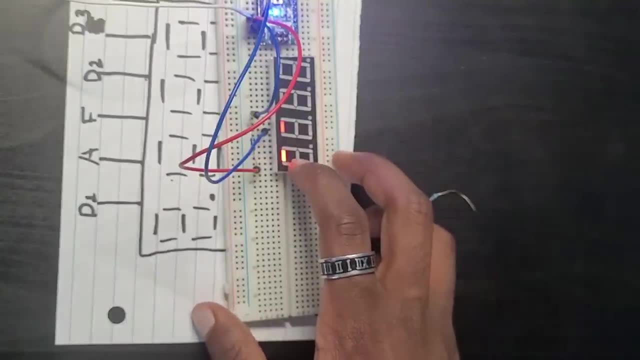 this one too, so they'll start copying each other, which is going to be bad, okay, so this is where the problem arises. okay, this is problem number one, the problem number one being what it copies the same thing. and the second thing you can see is, if you focus again, is the what, the division of 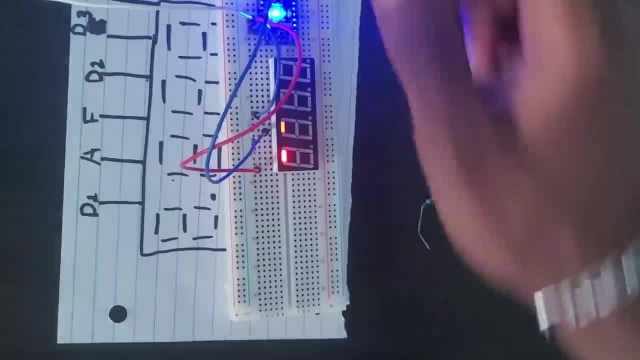 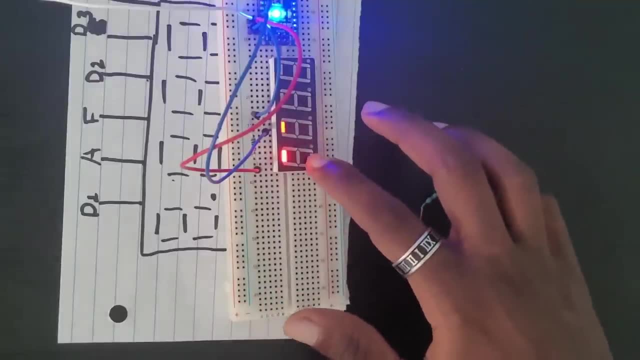 power is not very, very consistent. look at it. let me just turn off the light. one is very, very bright right here and this one is very dim now, just thinking, just think of trying to light up 32 different segments here, which is going to be what? almost impossible. it just even. 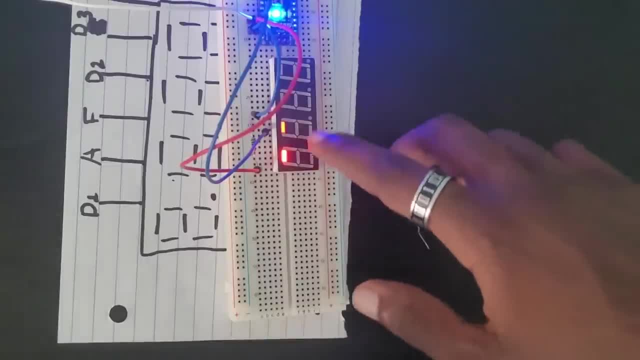 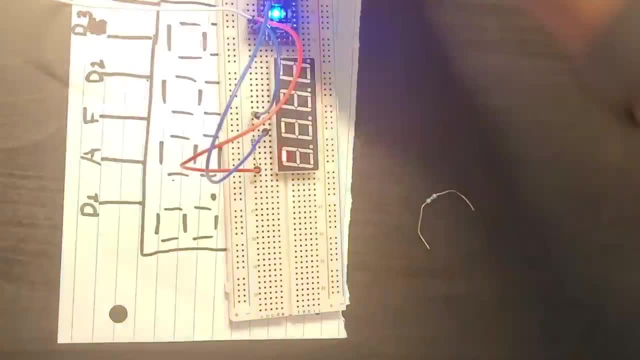 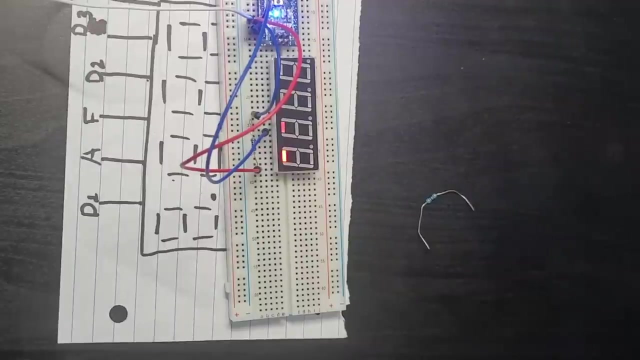 tapped out when we tried to connect it to an f, as you could. as you could have seen in the, when i tried to connect to f, right here the f pin, what happened? i just tapped out, it couldn't do it. basically, all of it turned off. okay, so this is the second problem that we have here. okay, so 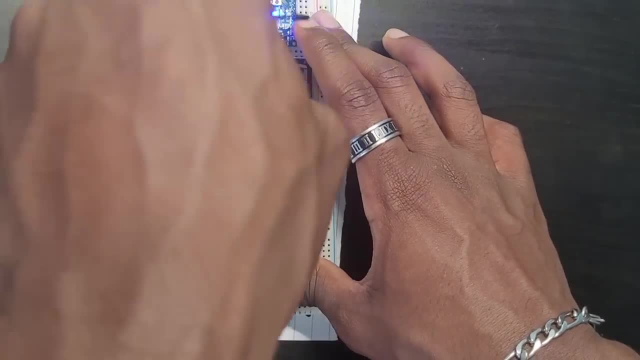 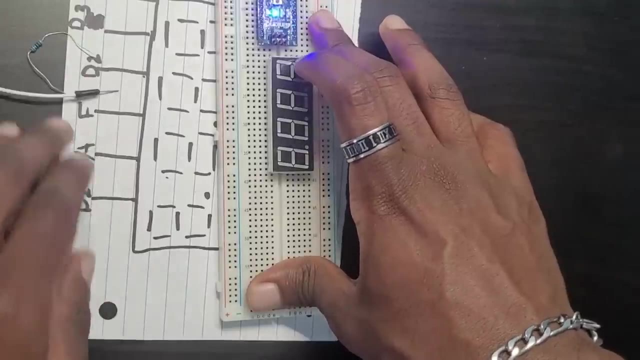 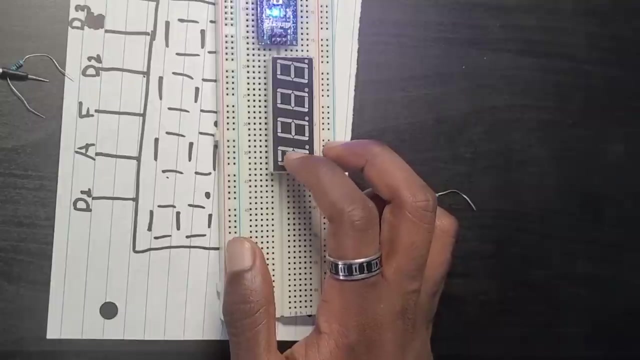 we're supposed to light it up, then well, one thing that you need to keep in mind is: we are always supposed to light up. just actually take off all of this. we're supposed to light up what we're supposed to light up- only one digit at a time, so we only can light up one digit at a time, so right. 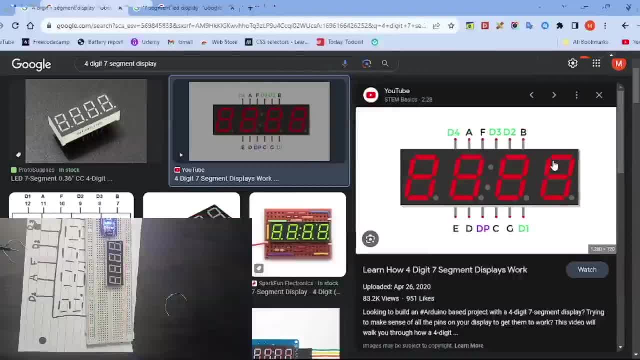 here. if you look- let me go again to the image right here. if you go to the image right here, what you can see is what a, f, b, all these segments are, what they're common to, what they're common to the d pins. the d pins are the ones that are specific. right here we have d1. we 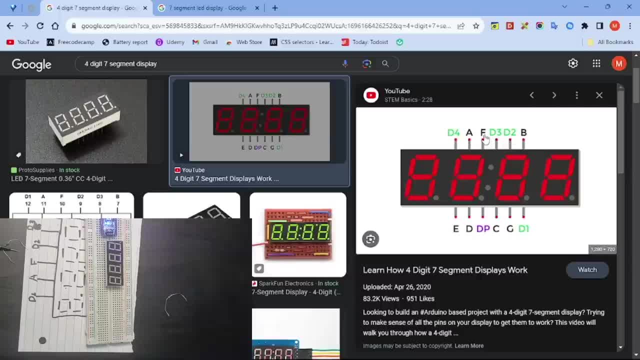 have d2, we have d3, d4- they're specific- while a, f, b, again e, d, decimal point, c and g, those segments right here, they're what they're common. they're common to all of them. okay, so one thing you can do is what we can light up everything here from a, all the segments. but we can do it. we're limited. 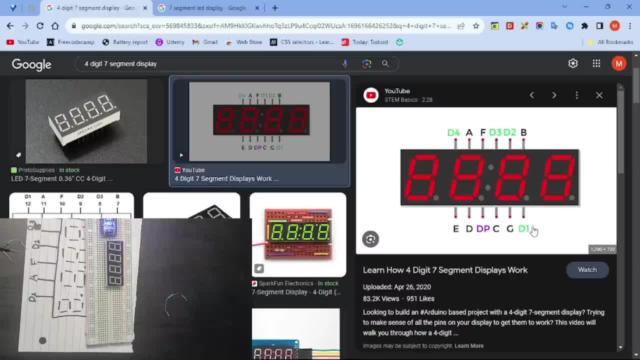 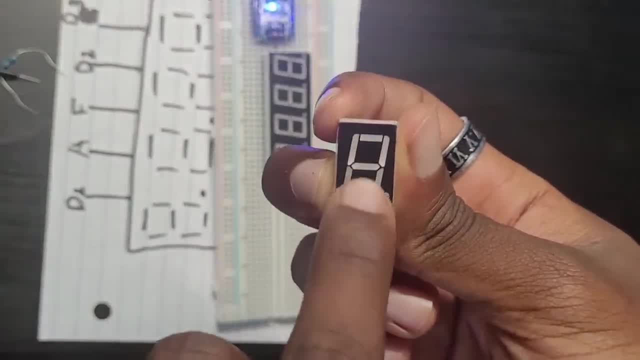 to what we're limited to. we're limited to one digit at a time. okay, we're limited to what? to one. so right here, when we do that again, when we just think of again using the one digit LED matrix, it's going to work perfectly fine when we're using one digit, I just want you to think of them as what is. 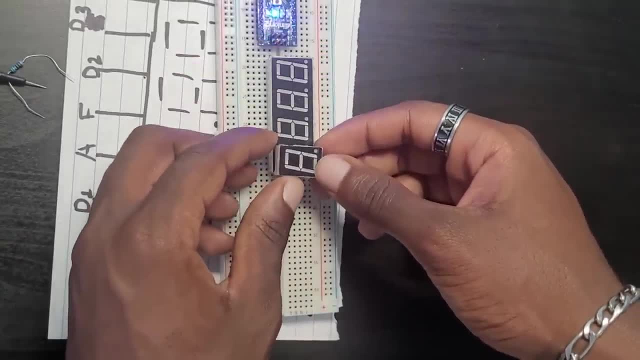 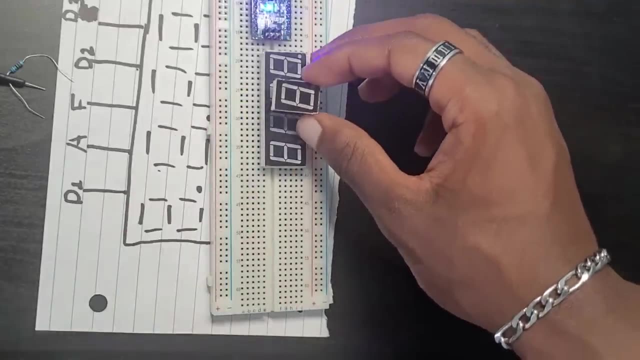 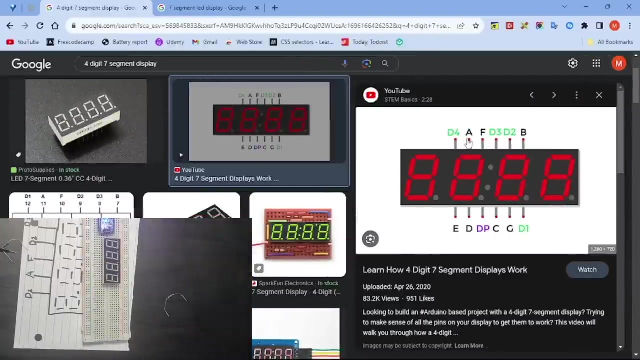 like four again, these four, what? these four one segment LED displays connected together, okay, systematically, so that they have 12 pins. so I just want you to think of them as what is? four again, four one digit seven segment LED displays. okay, so right here again. if there was specific we had, 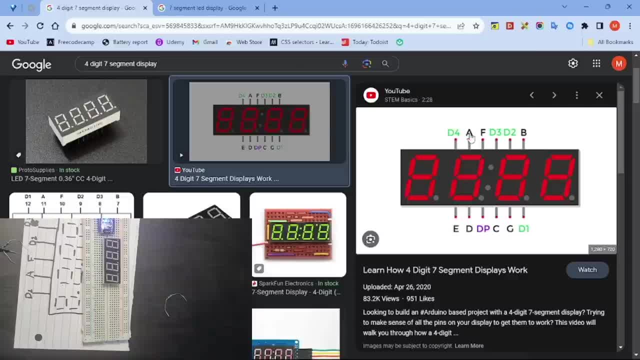 we have specific segments for all of them would be like a1. there will be a1. it will have a different pin for a1. we're gonna have a2, we're gonna have a3, we're gonna have a4. so basically we're gonna have. 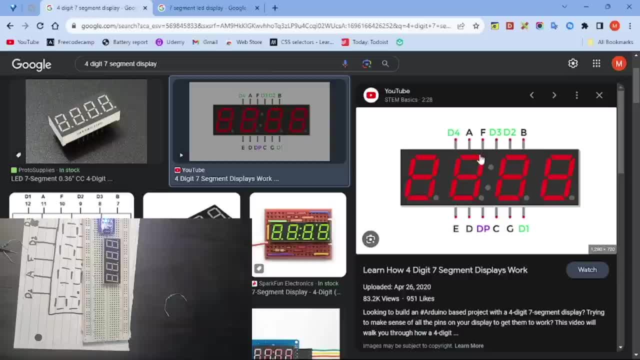 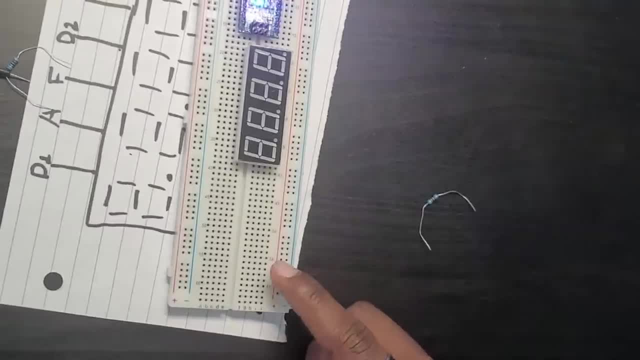 a lot of pins. obviously, you cannot work with all these pins, so another problem arises while using this method. the problem is okay. I want you to keep this in mind. the problem is okay. one digit at a time. okay, one digit at a time. okay, it works perfectly fine when we use one digit at a time. 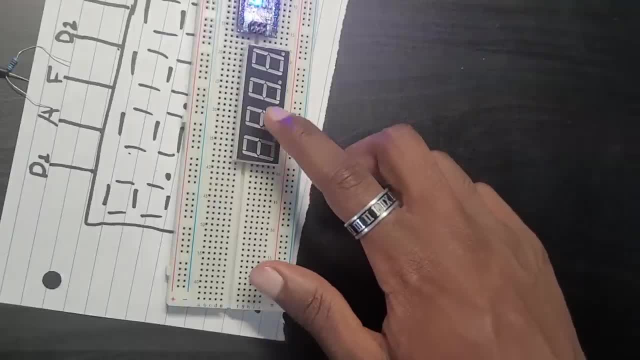 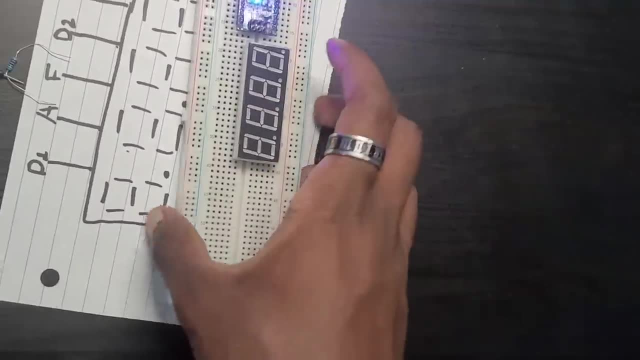 let's connect. uh, let me just connect three pins using the let's use digit number, again digit three, right here. I'm just trying to connect again just three or four uh segments right here. let me just do that so you guys can understand it. all right, let me just unplug this. where's my digit number? 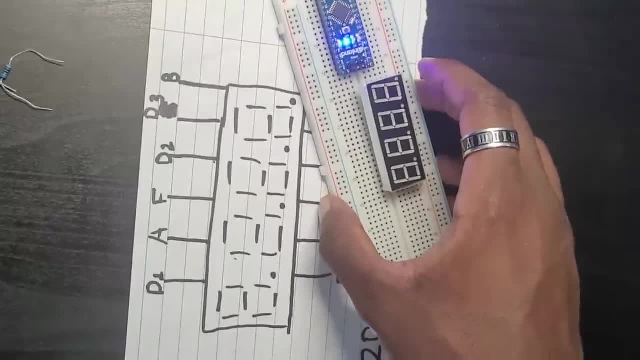 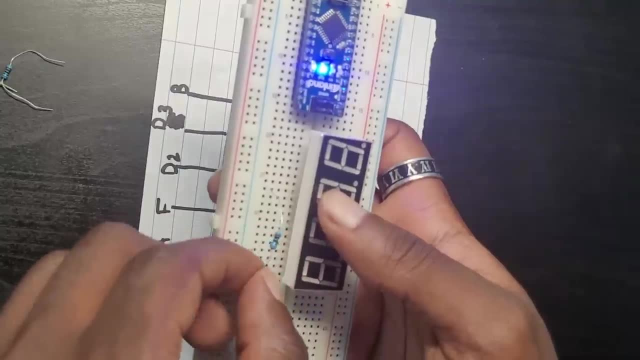 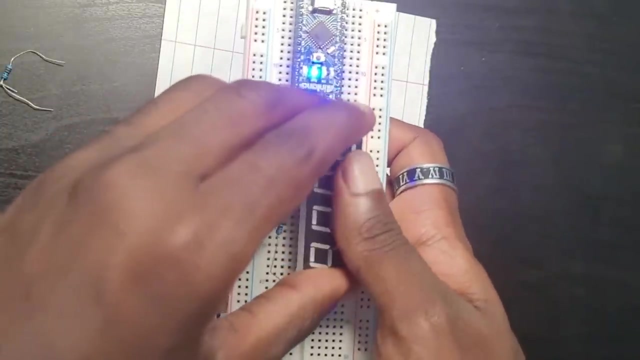 three right here. just number three is here. let me just focus here. digit number three is here, so it's going to be the one at the very edge, the one close next to the very edge. there we go, just push. let me first push this one so that it doesn't move a lot. there we go, but it's still visible. 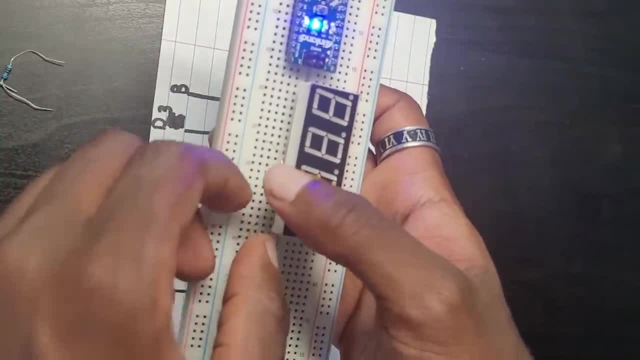 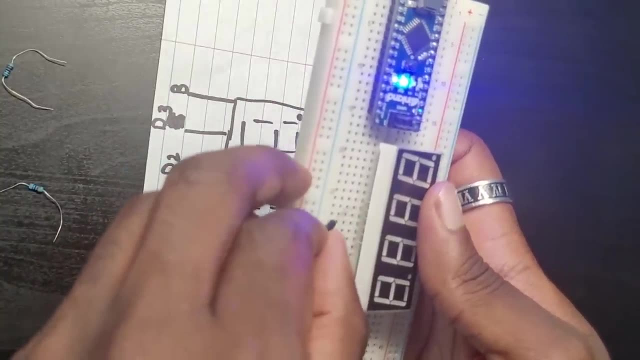 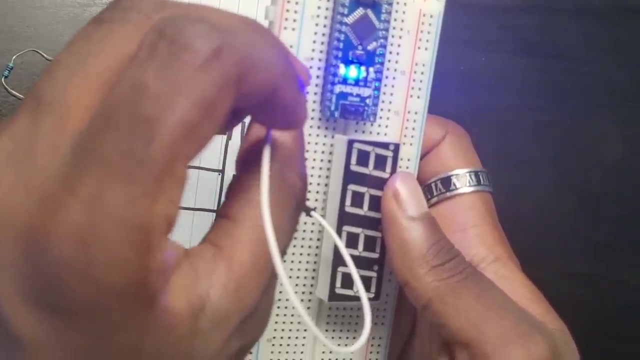 there we go. it's a. I'm lighting up what a digit. so I don't need to use my resistor. I'm just going to connect it directly to what. I'm using- a common cathode, as I said again. so I'm going to be connecting it to gnd. the d pins are going to be connected to the gnd. I just want you to think of. 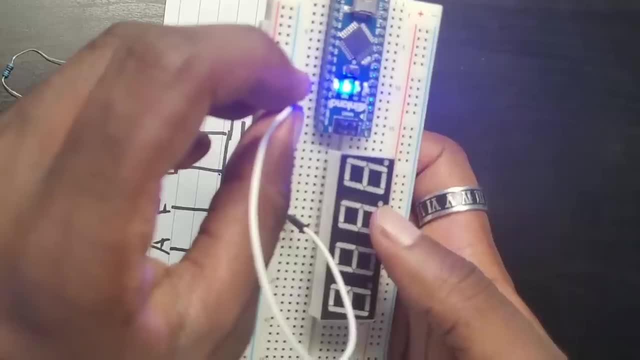 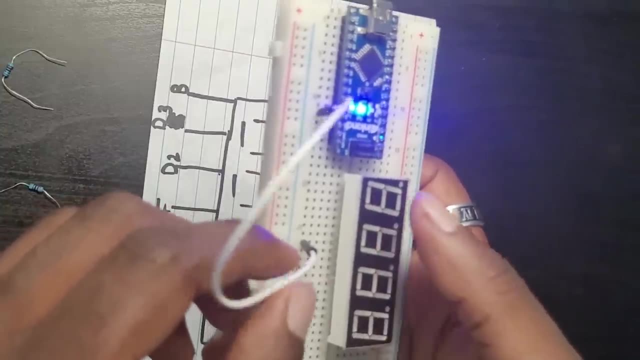 the digital pins, the deepens the sorry the. the digit pin says what I just want to think of them as common bits. again, they're marked with what they're marked with the number of their respective digit and like that they light up. okay, there we go. connected it to what I'm supposed to connect to gnd. there we 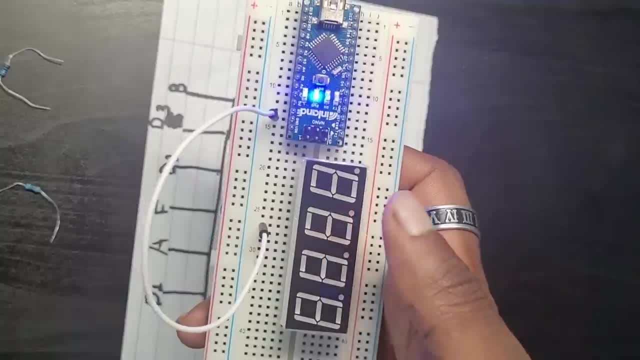 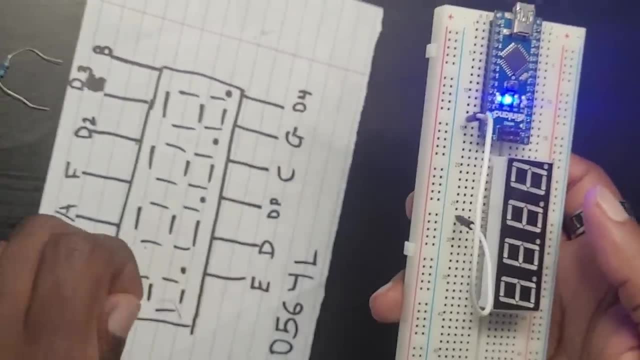 go connected to the gnd right now. let me just focus here so you can see it way better. there we go, and now what do I need to do? let me just light up again one segment right here. I don't care about that much, so okay, I'm just gonna light up B because close to uh, it's very close to uh. 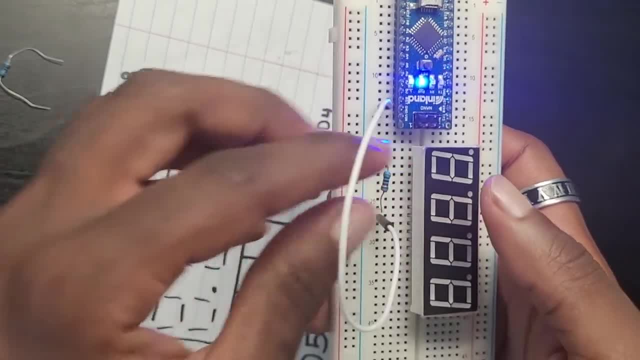 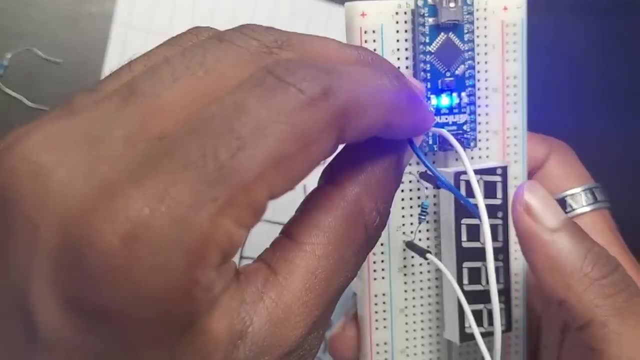 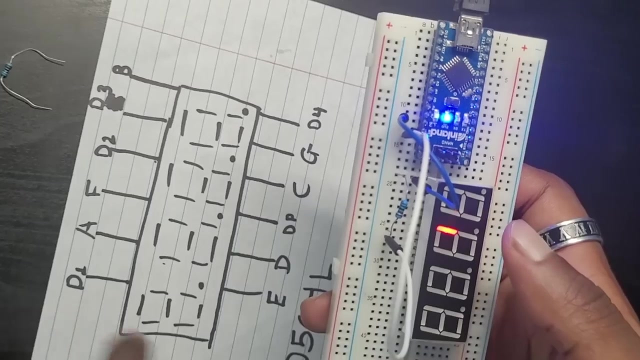 the digit number three. all right, there we go. now I'm just gonna need my wire. let me just wire this up and get my wire right here, then I'm going to be connecting it to the five volt. I've got my resistance all right. my resistance is: check. does it light up B? I think it lights up B. there we go. 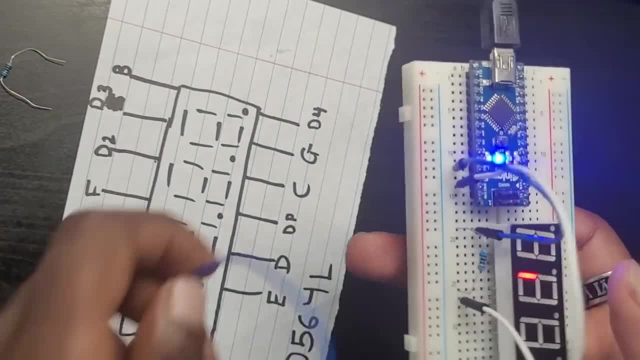 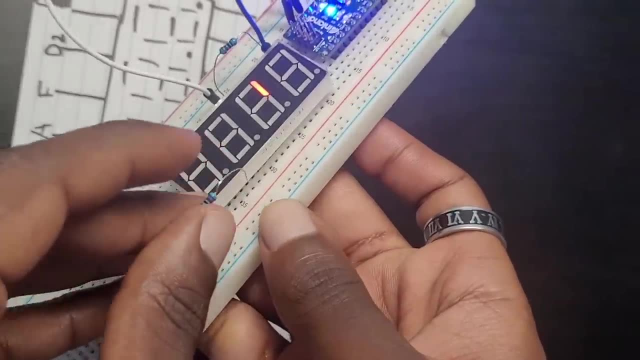 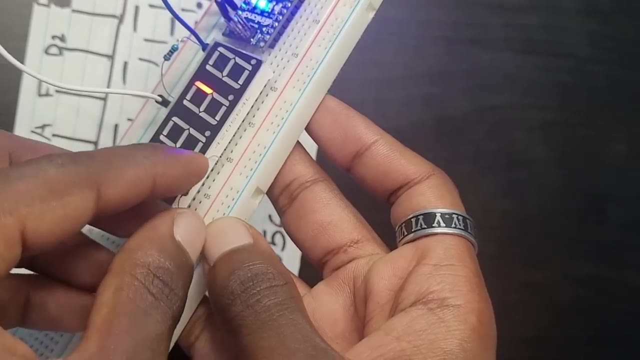 let me just try to light up another one too. just for the sake of it, let me bring another resistor. let me just light up someone that somewhere, that is here, let's go right here. can you see it? hopefully you can't. there we go, there we go, should be around. 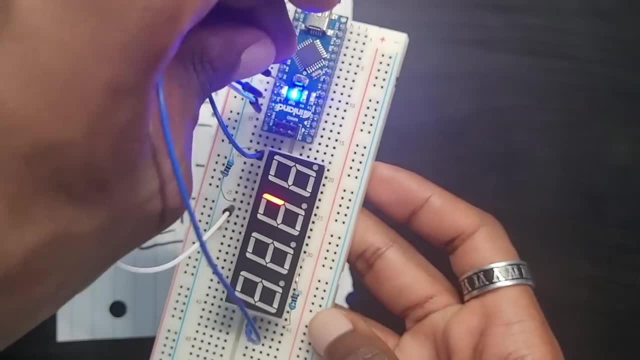 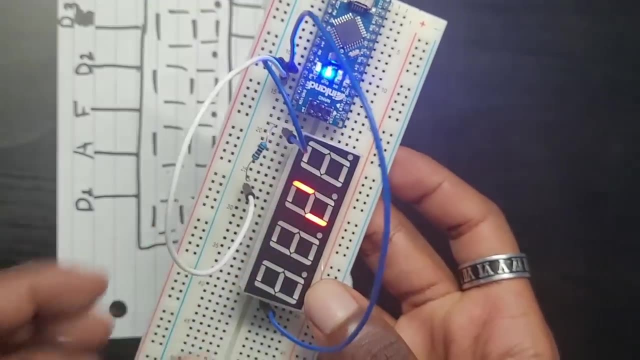 here. I'm going to connect this to five volts. let me just light up two. I think two proofs the point, so I don't need to light up more than two. there we go. okay, I need to push in the resistor. I'm just pushing this display and the resistor. 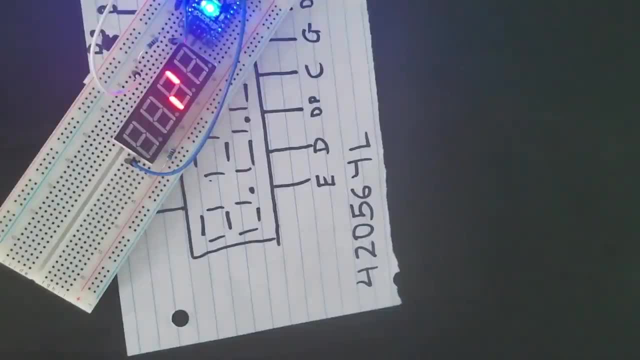 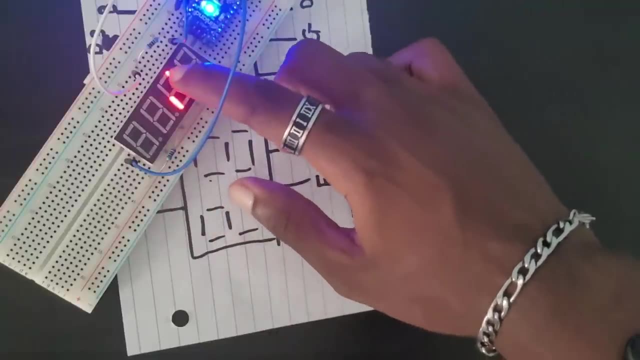 can you see it? let me again turn off the light. when we again use one digit at a time, what happens? what can you see it? it lights up properly. there is no what. there is no div. when you see the power division of power. right, there was uneven, right. 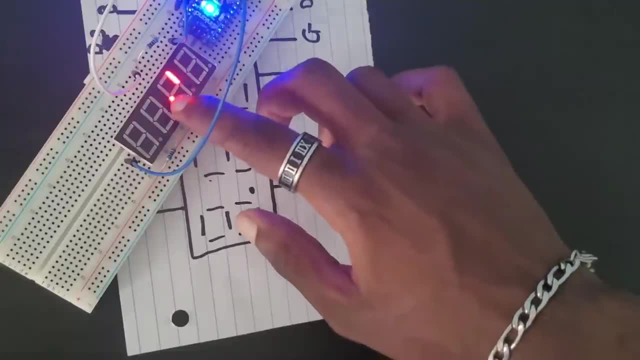 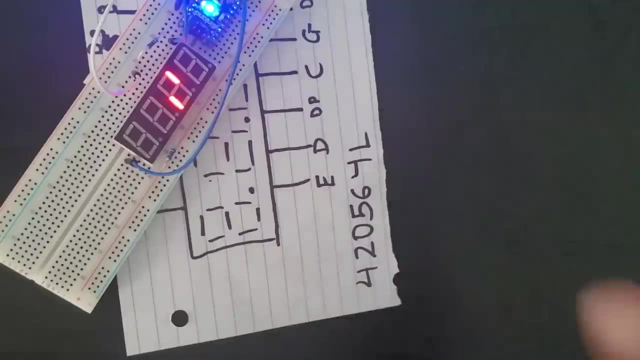 here it's even. okay, as you see it right. here it's even, and then two. I don't need to copy. it's not copying the same thing, but it rises again. another problem. the problem with this method is using one digit at a time because intended to do it's. because it's intended to be used at what? as one digit at a? 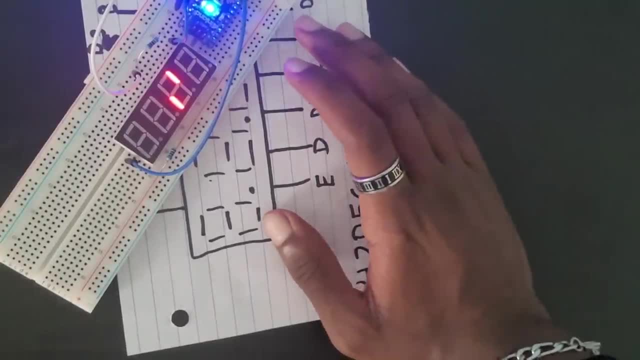 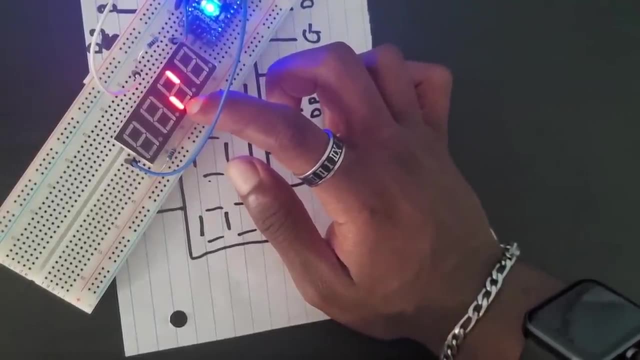 time. so what happens? here is the problem. most people, I think, think of our in nos. another problem is what if we use one digit at a time? it destroys the purpose of what. it destroys the purpose of having a four digit LED display because right here, let's see, we want to turn on, you know one? 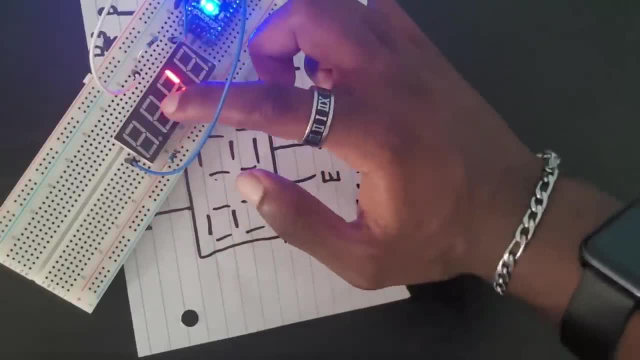 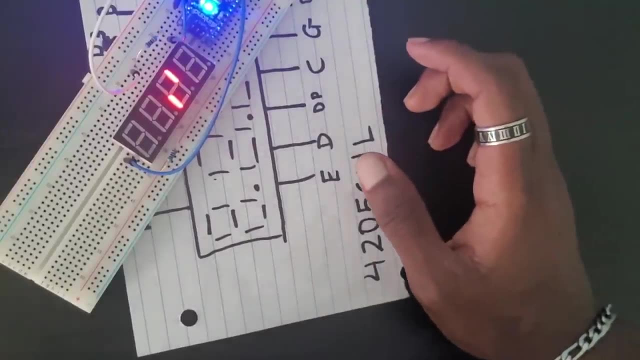 two, three, four. right here, it just starts to resistor. okay, let's see, we want to turn on one, two, three and four. right here, we want to turn on one, two, three, four. we can't do that if you're using what? one digit? one digit, um, they're only using one digit at a time. basically, what happens? 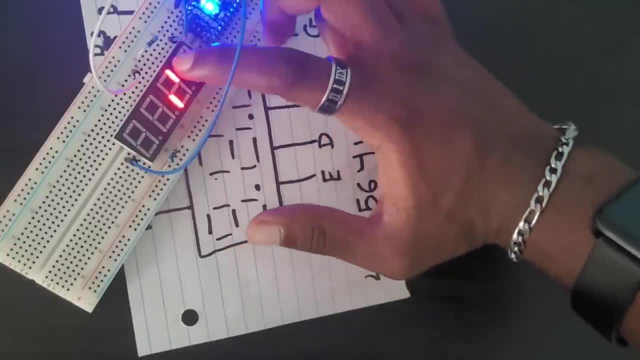 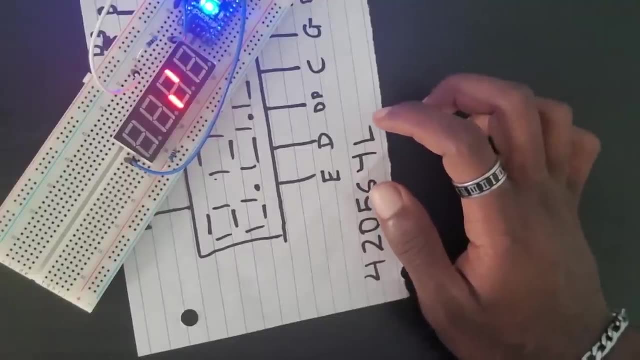 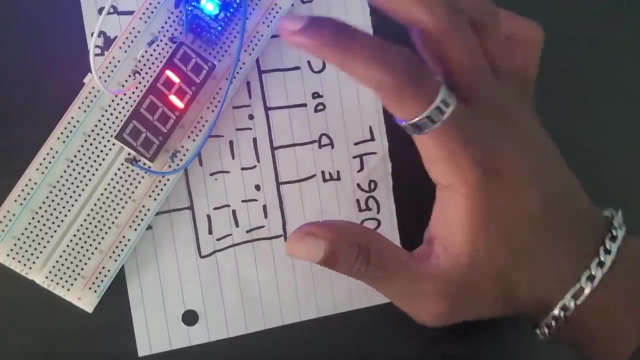 is one. what basically happens is what: we cannot turn on all of them at once. well, one thing i want you guys to keep in mind is: okay, um, one thing i want you to keep in mind is always is that these things are very, very fast. i'm talking about these. leds are microcontrollers. computers are very. 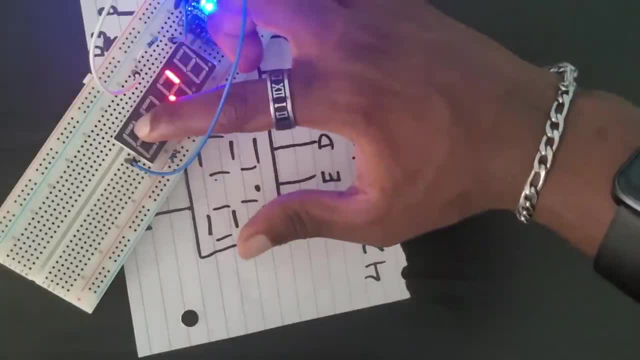 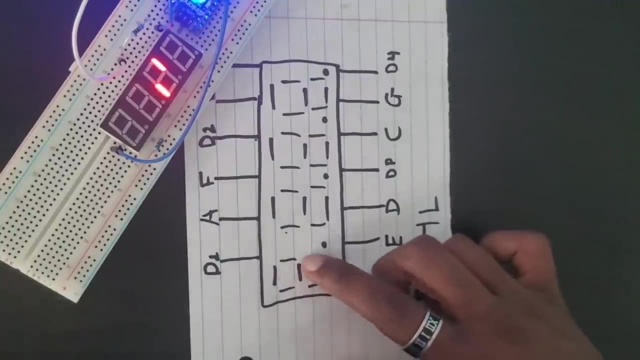 very fast, okay. so let's say we want to turn on one. where do we go? we go to digital pin one and then we turn on again two segments. we're going to turn on these two segments. okay, we want to turn on let's say one, okay, one, turn on that. and let's say we go to additional. again, we're gonna go to. 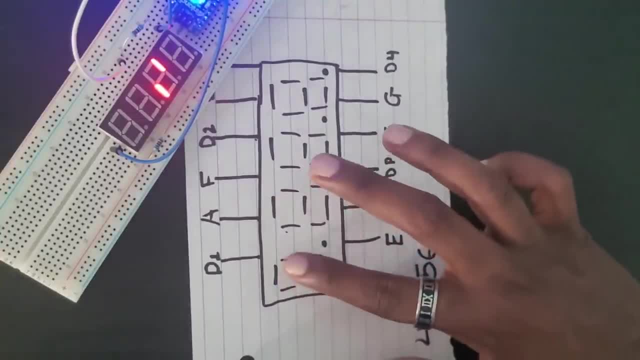 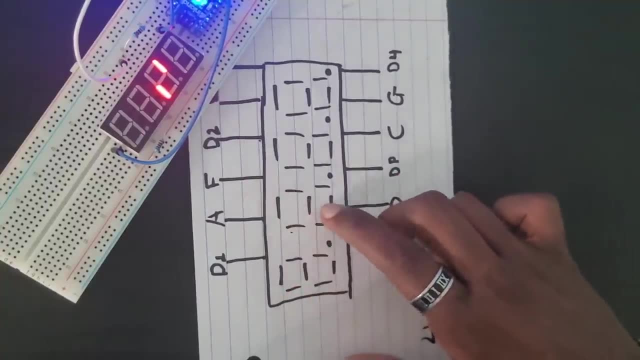 digital two. we're gonna turn this off after we're done with it. we're gonna turn it off and there's still pin two. we're gonna go to d2, connect d2 right here and then we're gonna light up all these segments again. the one that marks a two, we're gonna go right here and light up all these. 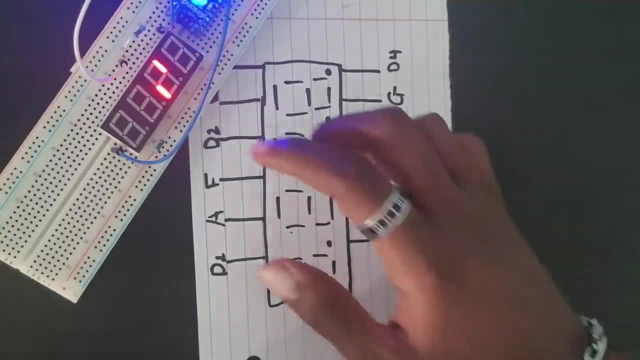 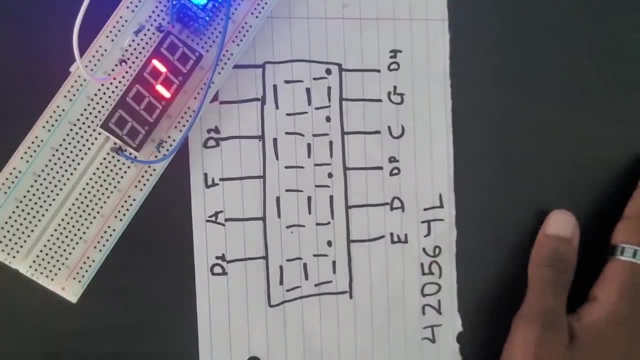 segments right. so you might think that it's gonna go really slow. we're gonna see one right here and then we're gonna see two, but it's gonna happen very, very fast. okay, i'm talking in milliseconds. it's gonna happen very, very fast in milliseconds. that we're not 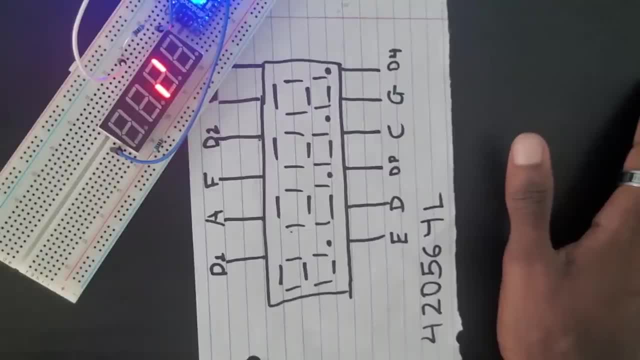 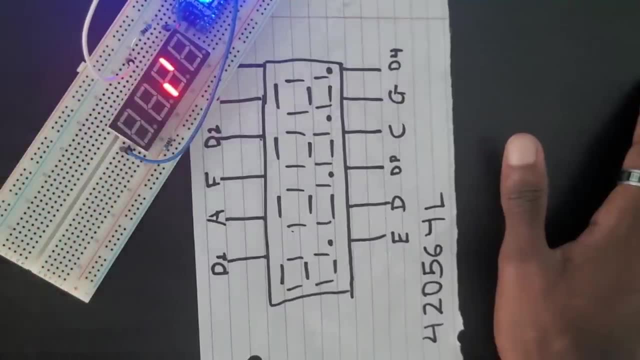 gonna notice one turning off. okay, we're not gonna notice one turning off and then switching to two. one turning off right here and then and arduino going here and lighting up two. it's gonna happen so fast that we're gonna what. we're gonna keep seeing one and then we're also gonna keep what. 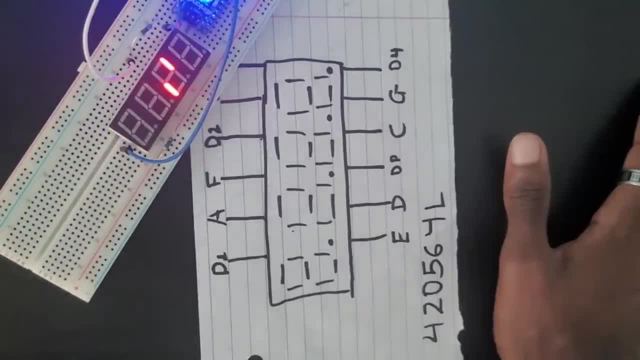 seeing two right here. okay, for our eyes it's not what it's not visible for us. so that's one thing i want you guys to keep in mind. we're going to be lighting up one digit at a time, but it's going to happen very, very fast that our eyes cannot what our eyes cannot notice it. okay, our eyes cannot. 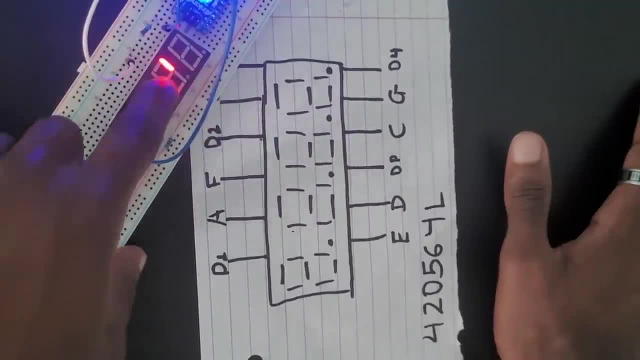 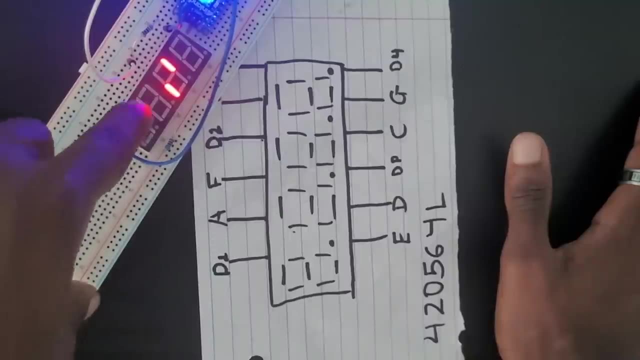 notice it. so that what? so that we can basically what? turn on all of these at once. so we can turn on all of these at once. so, technically speaking, we're not turning all of these at once, we're turning this on, we're turning this off. once we're done with this, we go to this one and then once. 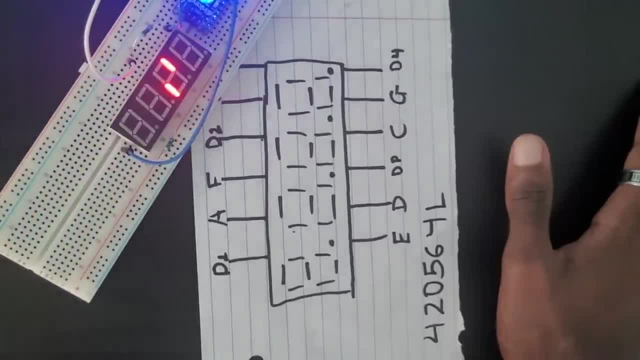 we're done with this, we go this one. once we're done with this, we go this one. but it happens very, very, very fast that our eyes cannot notice what- this turning off, okay, these turning off, okay, the others turning off- it's going to happen very fast that all of them for us. 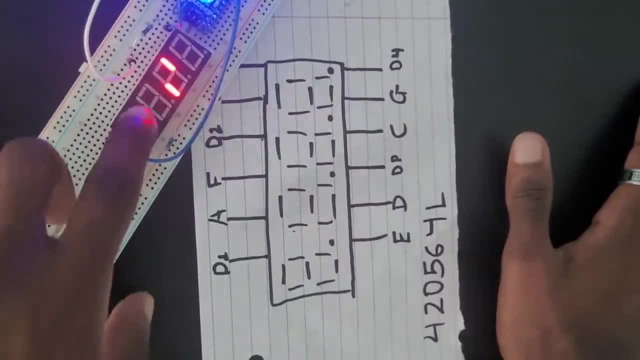 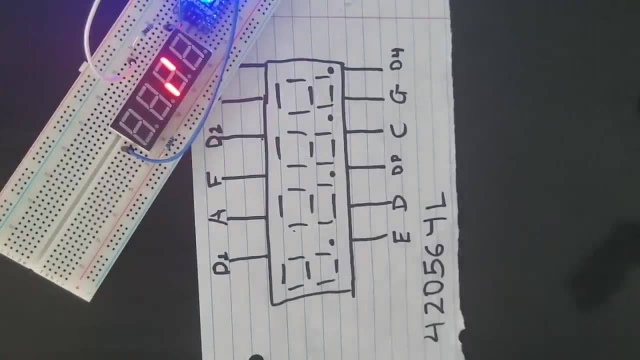 it's going to appear that all of them are what all of them are on, and they're what they're displaying, what they're displaying numbers. okay, that's one thing i want you guys to keep in mind. okay, so right here. one final thing before uh, moving on is again, the problem here is what let 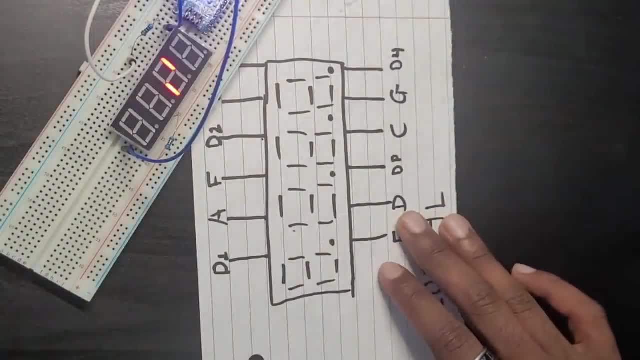 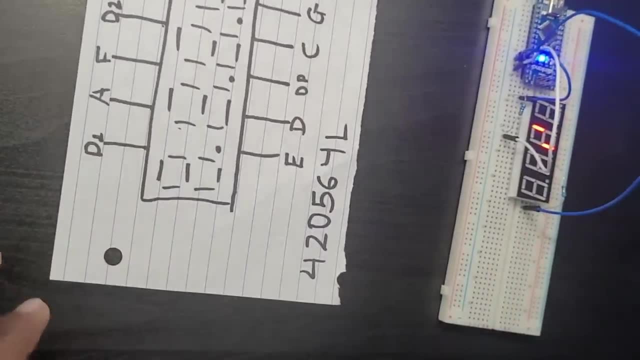 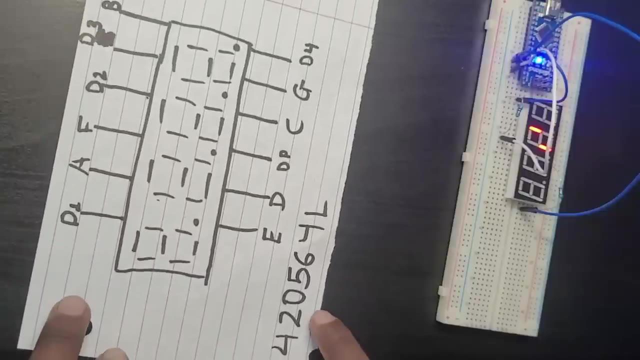 me just turn on lights. the problem i encountered myself was: okay. the problem i encountered myself was i could not find the documentation on my specified type of what? on my specified type of four, four digit uh seven segment led displays. okay, i could not find specific data sheet. okay, if you look at the image right now, when 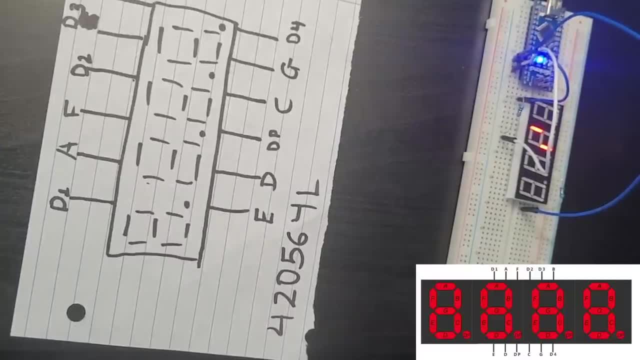 you look at the image, it's very, very different from my one. it's very, very different from the one that i have here. almost everything's the same when it comes to segments right here, a, f, p, e, d, d, p, c and g are the same, but, uh, but the layout of the one, the digits, is very different. digit one right. 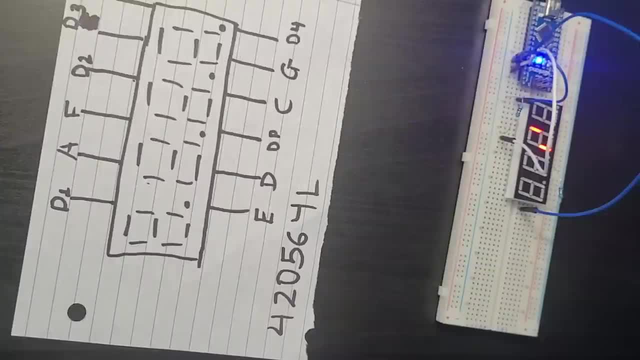 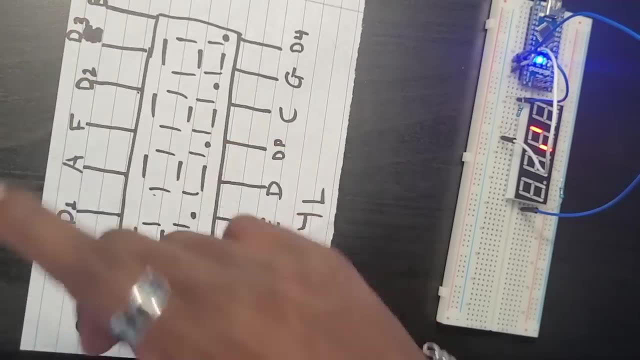 here is located at the very, very left for me, left top, while digit four and that well in the image. so again, how do we find you know which is which and how do we label them and write this down for ourselves, because sometimes you might find what if you have a less popular? uh. 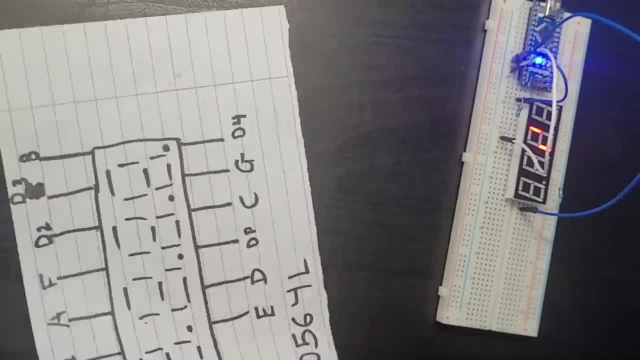 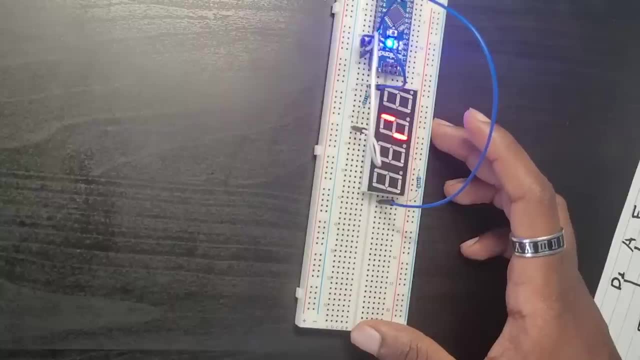 less popular type of code. right here you're not going to find what you're not going to find: your led display dd sheet. there's a lower chance of it because i did not find it myself. i've been looking around for like a good 20 minutes, 30 minutes, but i could not find any data sheet. 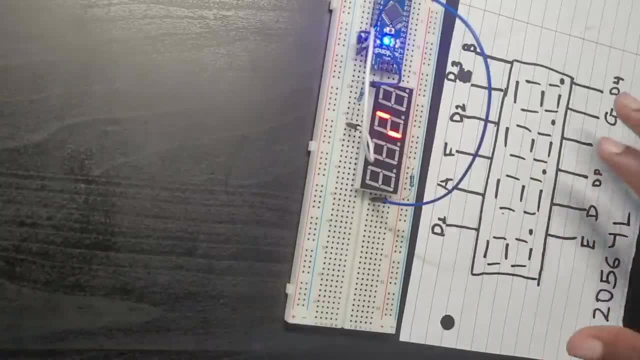 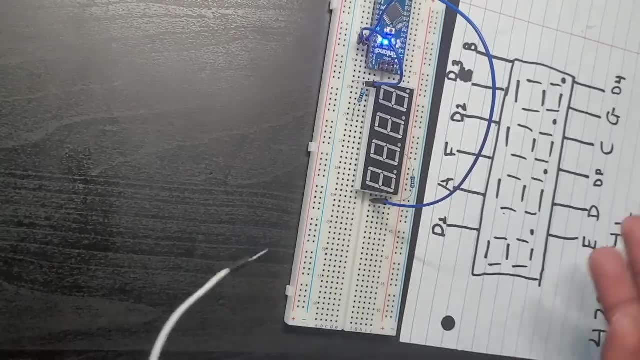 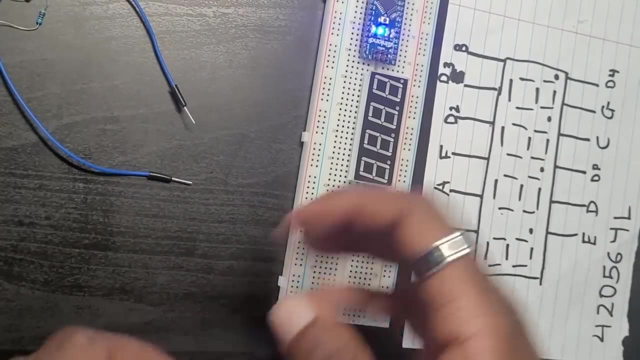 on my specified type of um four digit um semi-segment led displays. so right here, what i did is i wanted to know if it's a common anode or a common cathode. okay, how do i know that? let me just again begin from. let me just turn all of this off. okay, let me just do that. how do i know that? 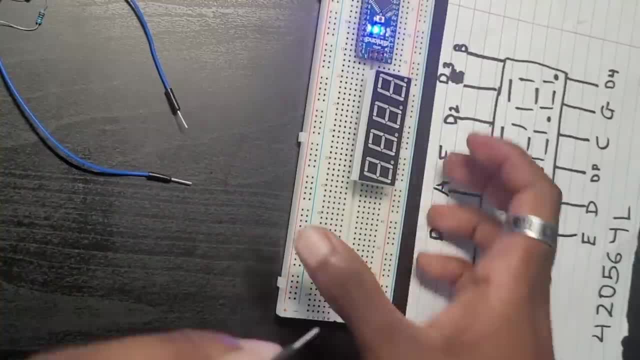 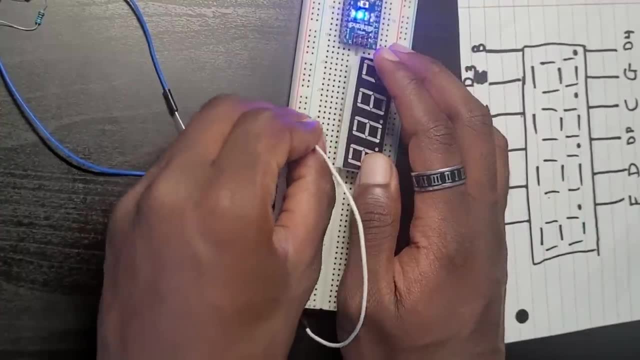 how do i know that? okay, how do i know that? what i did is what? okay, i just assumed that's what this is going to be the digit pin right here. let me just assume this is the digit pin. okay, again, assume this is what this is going to be: a digit pin. i just started with this and i started. 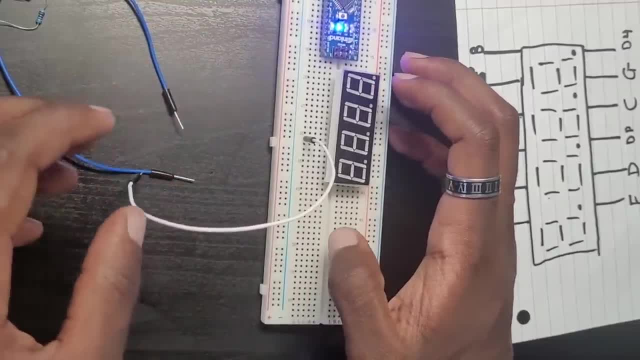 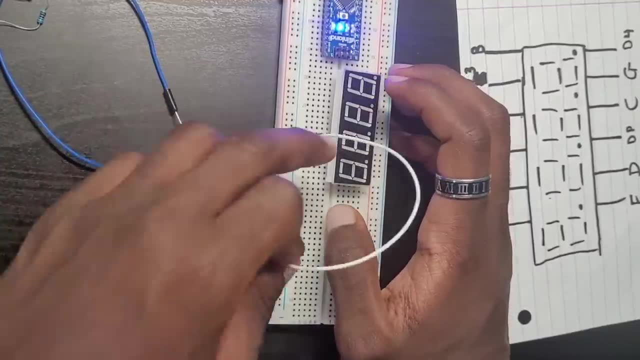 to what i just assumed. again, you're going to. you're going to be doing it with trial and error, okay, you're going to be using a method of what? trial and there until we get one segment, okay. so right here, let me just again use this as a what? as a digital pin. right here, i'm going to. 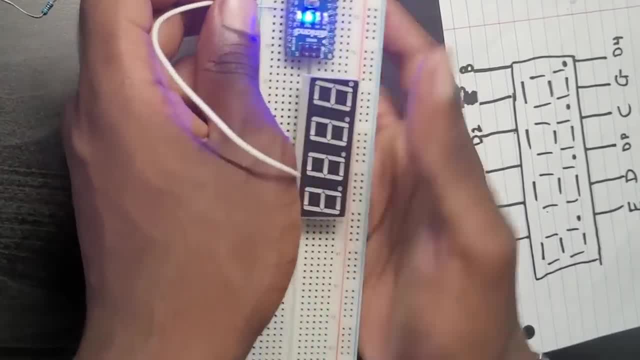 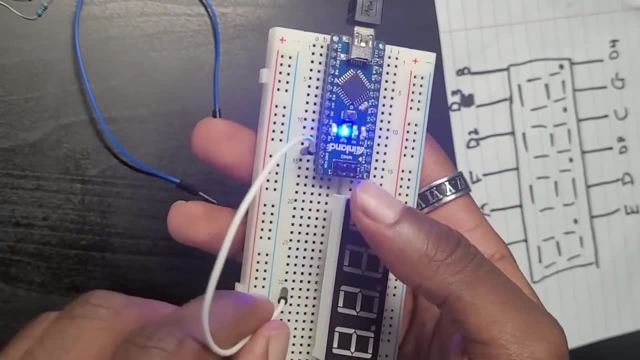 be using it as a d-pin, as a what i'm just going to assume. this is a common cathode, so this is a d-pin. what is it going to be? it's going to be connected to gnd. connect to gnd. all right, i'm going to assume the other one, the next that is right there as a segment again. 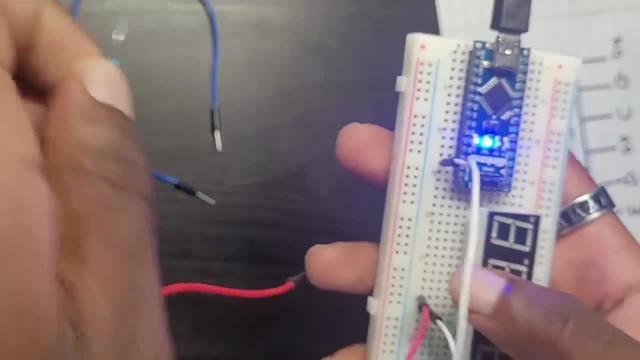 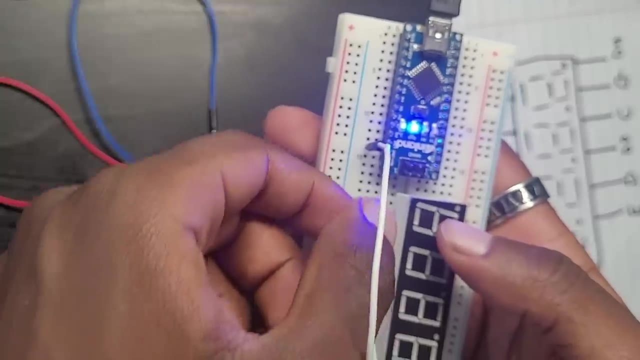 so you're going to keep on trying until again you find the right one, until you find one. uh, one segment lights up. okay, let me just again assume this is a common. let me assume this is a common. actually, you know what this is: a common cathode. but let me just assume this is a common anode, for 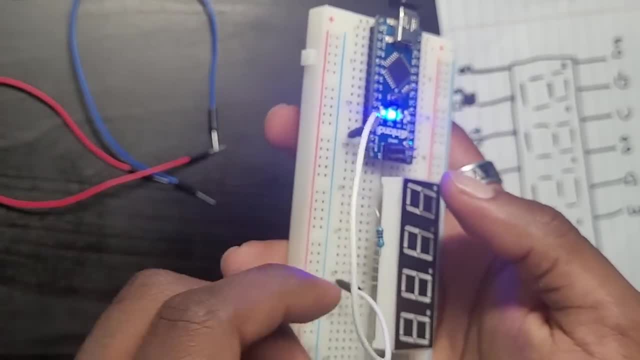 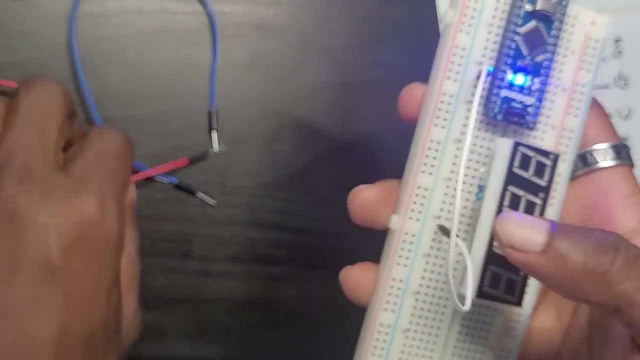 now. so to make things very easier for other people who have a common anode. so let me just show them right here. i'm going to be connecting this to the what if it's a common, and i'm going to connect 5 volt. let me just do that and let me bring another pin again. i have my resistor. i'm 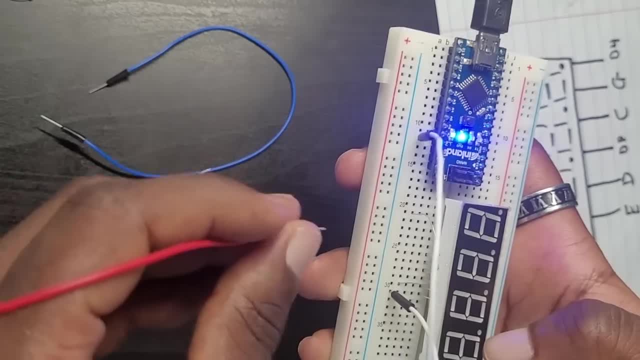 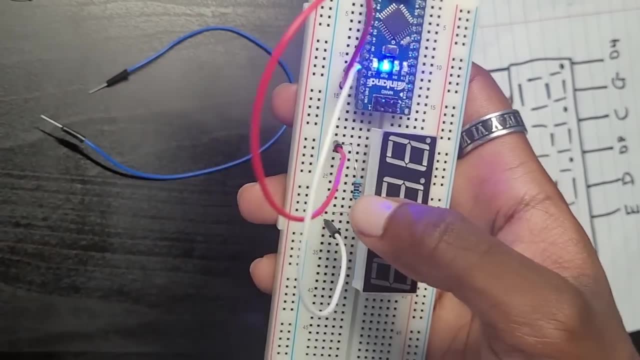 assuming this is what this is: a segment next to it it's a segment. i'm just assuming that again, this is assumption. until we find, until we basically what? until we find when it's right. always one thing you have to always keep in mind as well. you always have to light up again. 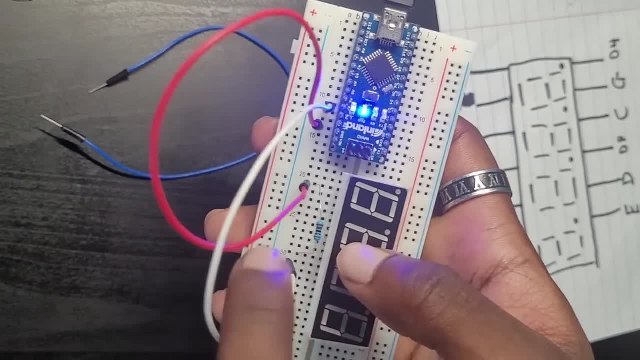 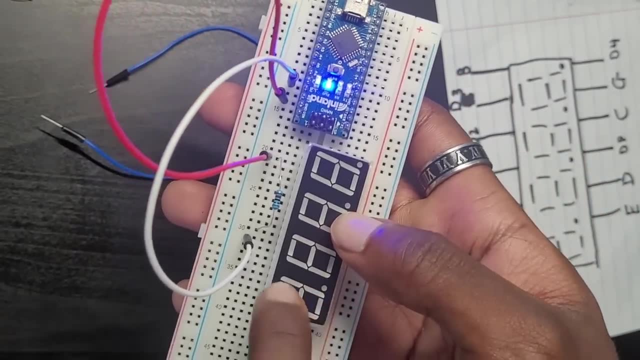 or what. we always have to use resistors, because if we try to connect one without any resistor, what's going to happen is when we're trying to find out which one's which we're going to basically what fry our leds, our segments right here. we don't want to do that again. 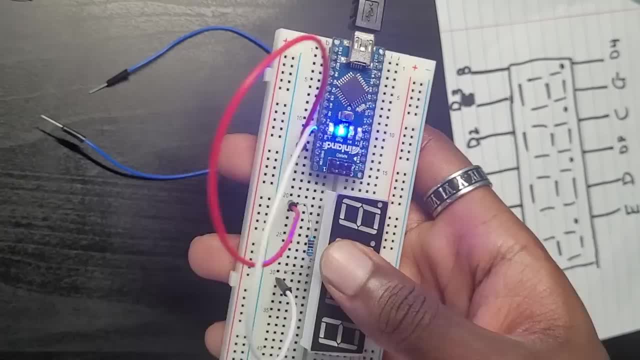 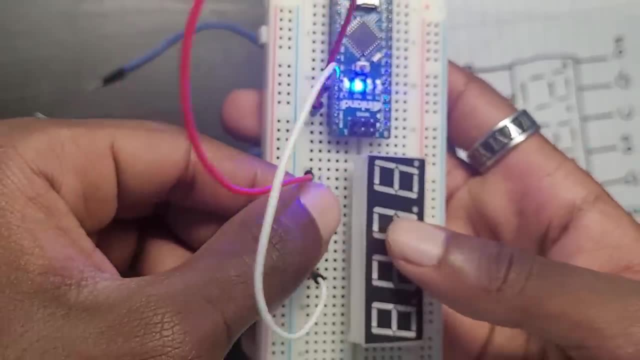 okay, so just keep that in mind. okay, it doesn't turn on. okay, what i'm going to do is i'm going to be moving. i'm going to start moving. okay, i'm going to be starting to move my resistor to the other pins. i'm not going to change the comment pin again, i'm just going to. 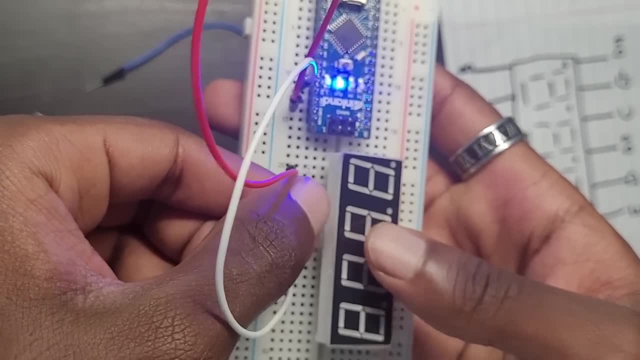 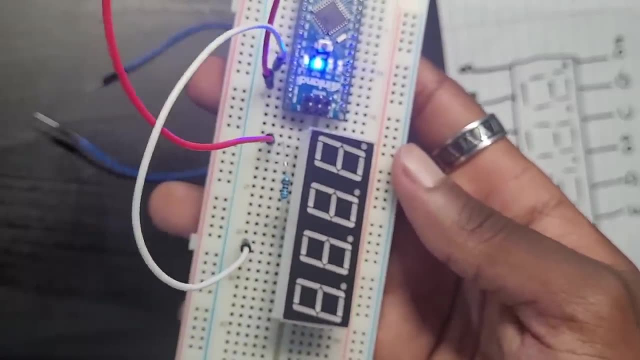 keep it like that for now. i'm just assuming this is a d pin. okay, i'm just going to keep doing it. let me go the other one right here. let me focus actually here. there we go, i'm just going to keep doing it. it's not lighting up again. pushed it, let me. 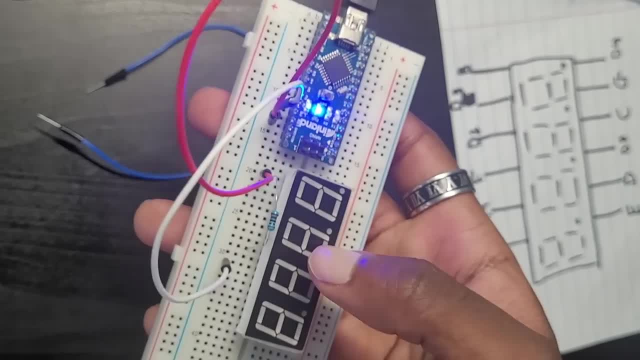 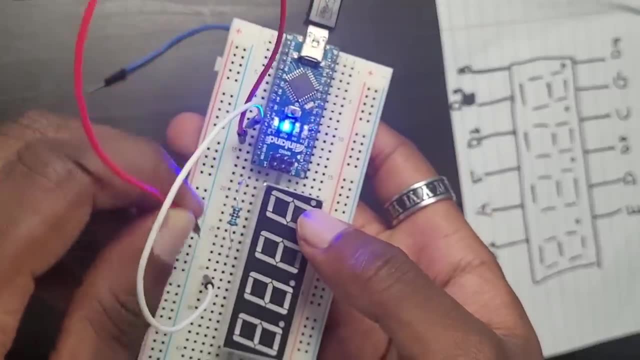 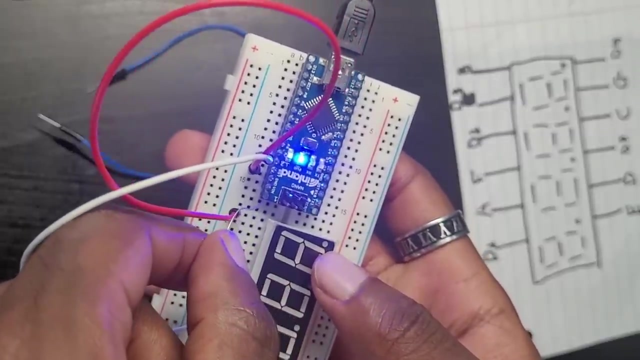 just push it again. let's push it so they can even see it. there we go. it's not lighting up up. i'm just going to keep on moving the resistor again, one one at a time, to the next pin. try to connect the other one. it's not lighting up. okay, let me try the other one. let me try a whole row. 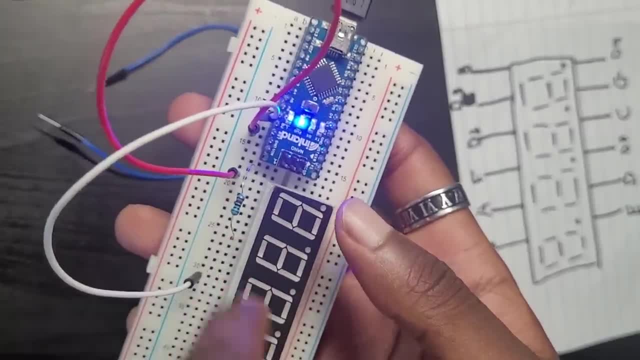 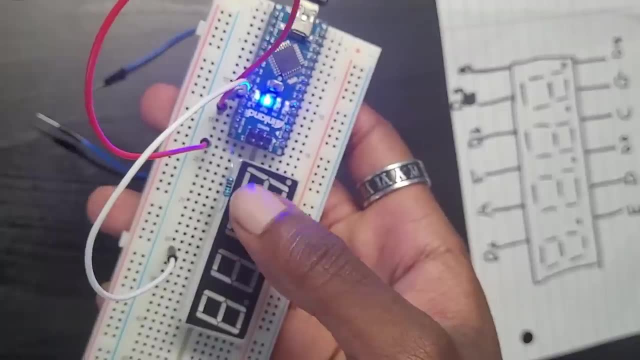 before actually concluding. okay, so let me try at least one of these six pins before actually concluding. so okay, let me just try to connect this one to the resistor. is supposed to be here. okay, it's not lighting up, so what could i possibly see right here either, i did not connect it to a 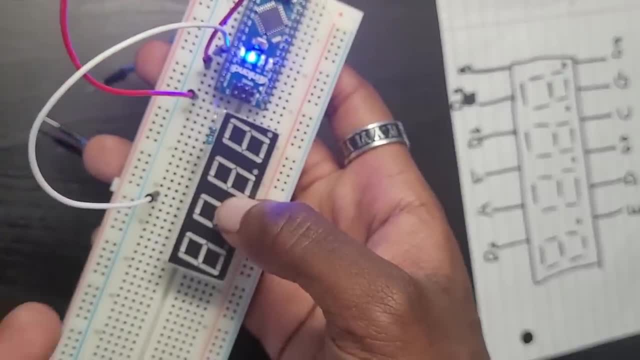 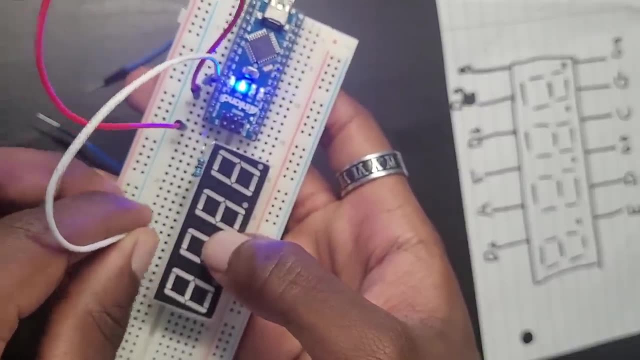 right, digital pin right here. so, okay, i do not know if i can connect this one to the other one or connect it to what, to a normal d pin. i'm just going to assume again a segment again. i'm just going to keep doing this until we find what a correct answer. so let me just keep touching this. 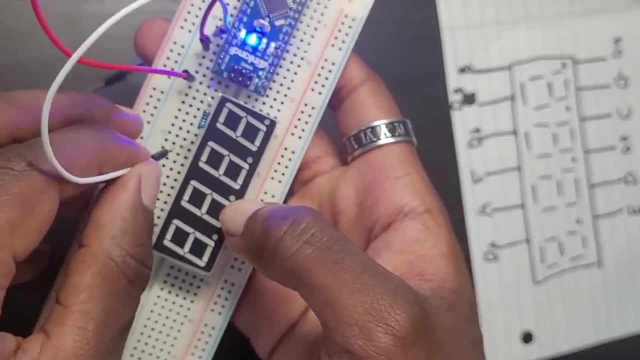 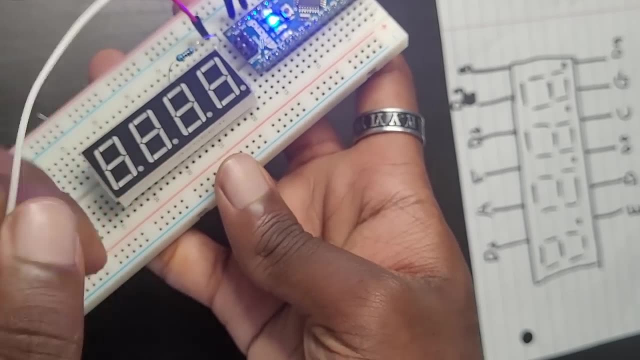 again changing it, keep changing it. okay, i reached the resistor point, so i'm not going to touch that again. there is a probability of finding it. let me go to the other side right now. now we have to find again one of those digit pins are supposed to be here. 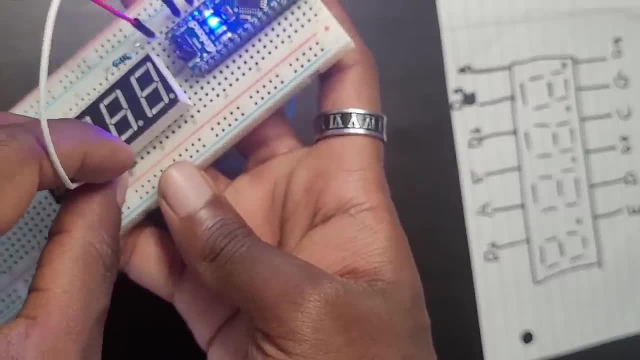 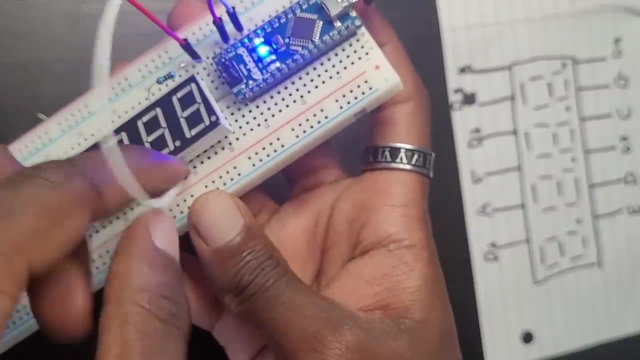 one of them is supposed to be what digital pins right here? just keep doing it. keep doing it. it's not lighting up. nothing is lighting up right here. keep doing it. all right, i reached my end of this side. so basically, what could happen is what i reversed it, basically so. 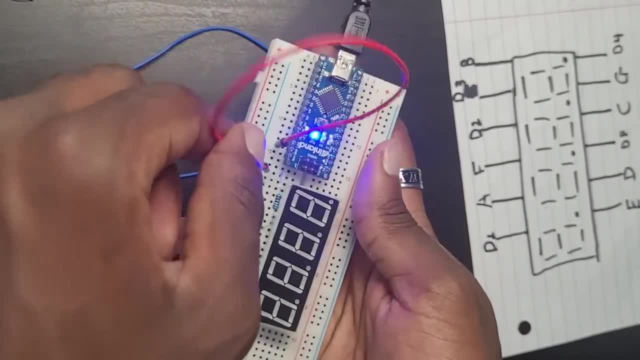 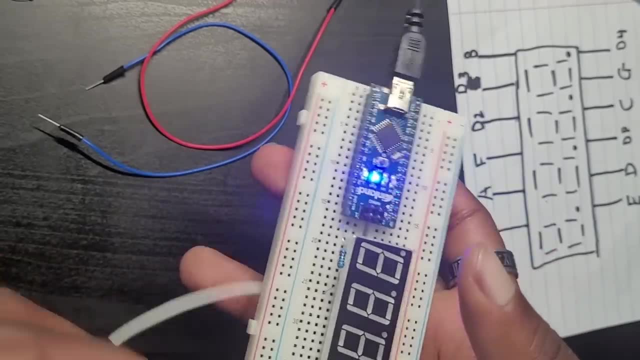 what it could be a common, what a common cathode instead of what a common anode. right here, i tried it as a what is a common anode. okay, it's not a common, what it's not a common anode. so let me try a common cathode. so let me just reverse it. so, right here, what do i need to do is again set. 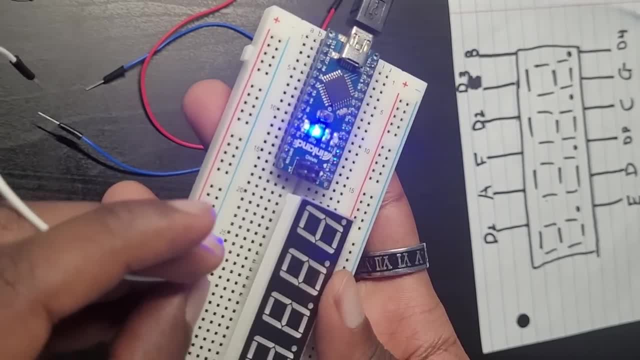 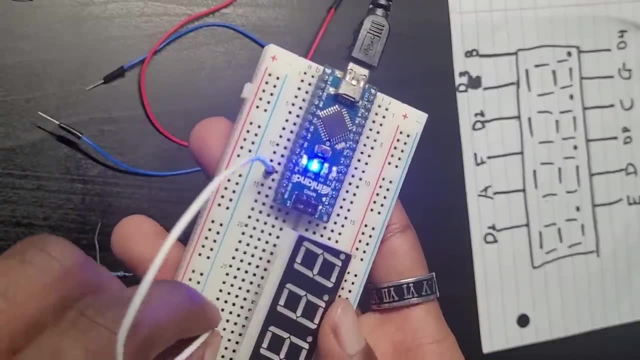 the card the d pins are supposed to be set to what they're supposed to be set to g and d. let me just do that again. so i'm going to be assuming this is what i'm going to be assuming. let me start actually from right here. keep on, let me just start from here, because i know this is the. 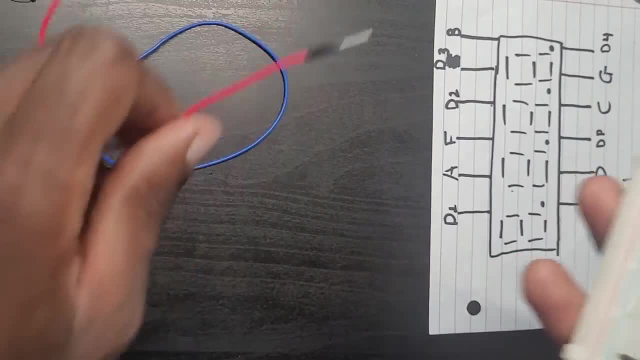 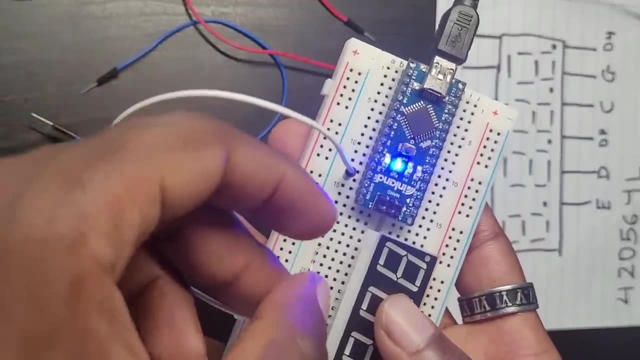 deep end. i don't want to start from here. i just want to show you guys how you do it right now, since i already wrote it down again. i wrote down the documentation. all right, let me again go here right here. let me just again put a segment right here. 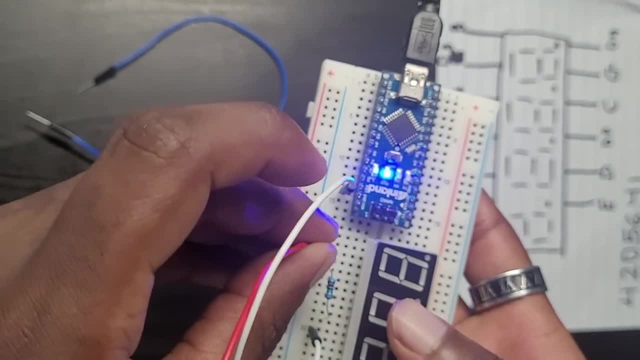 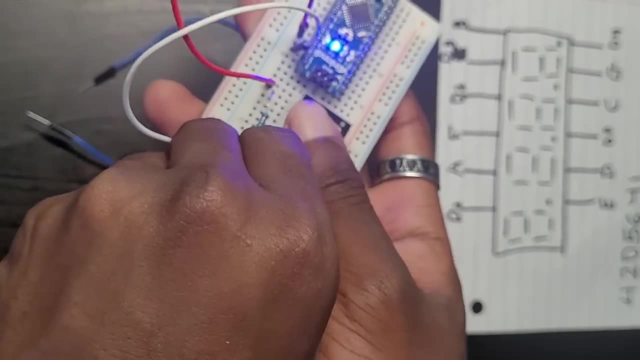 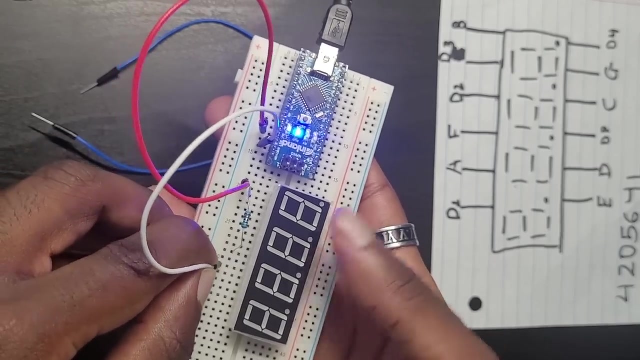 and let me connect it to a what, to the five volt segment, to the five volt segment, to the five volt. okay, let me again push it. push it a bit in so we can see it. there we go. nothing is lighting up. okay, maybe i have to move this again here. let's see if it lights up. where's the five volt? 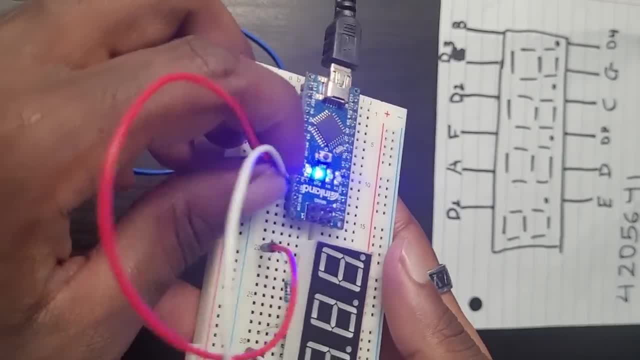 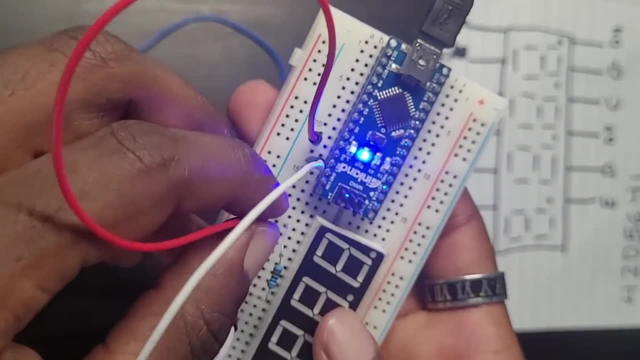 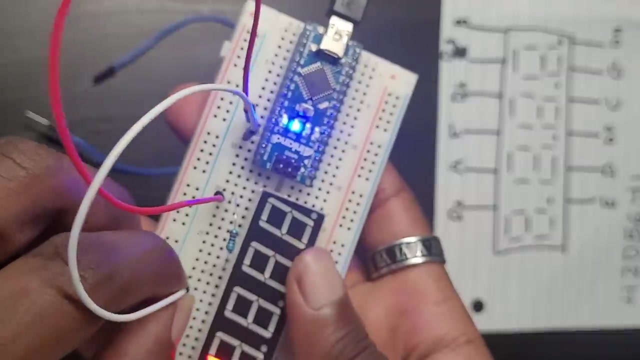 did i get the gnd right? i think i got the gnd right. um, wait, all right, there we go. oh, i don't know, i didn't connect this one to the proper resistor and i'm supposed to connect the same, the same row. there we go, can you see it? oh, now it's lighting up, if i put it right here. 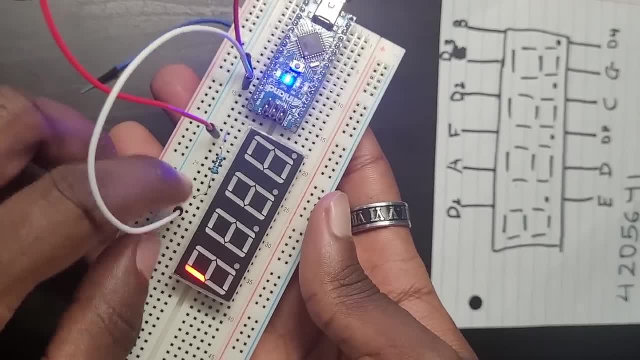 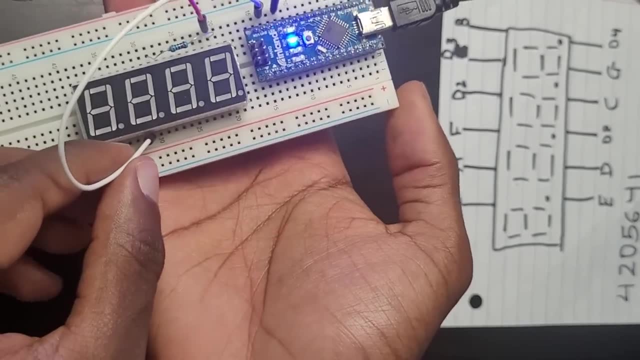 it doesn't light up, but if i just put it here it lights up. okay, let's say, i do not find this one again, let me just go over right here and let's try to find it again. let me just try to find. let me just try to what my objective here is: to at least try to find what. 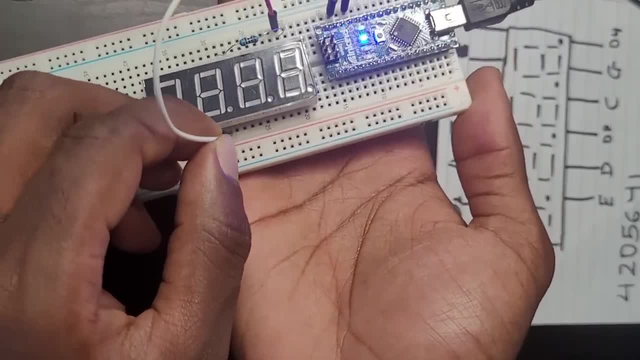 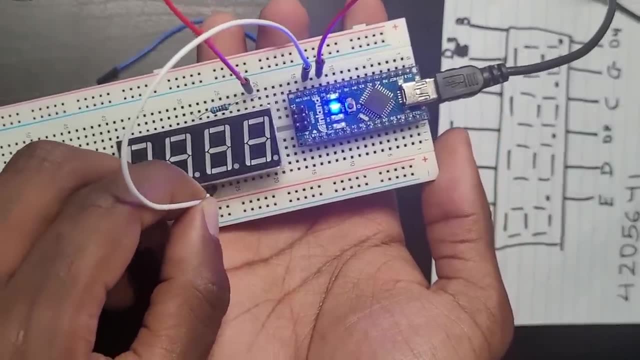 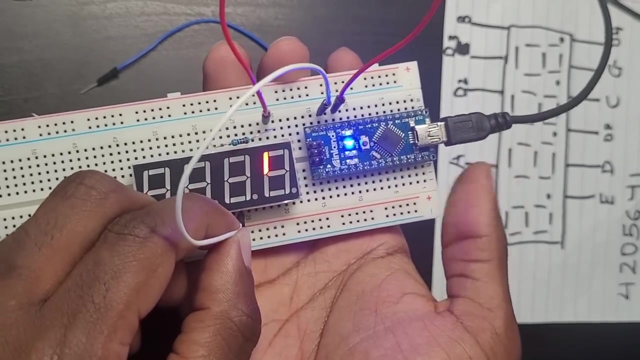 try to light up one segment. that's, that's my only objective here. as soon as i do that, it's going to be easy. oh, what did i do wrong here? let's keep on pushing it again. i'm just going to make sure the resistance is again intact. oh, now it's lighting up, so let me just say: okay, this, let this light up. 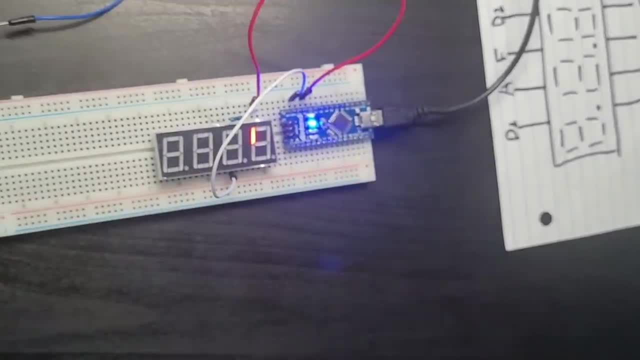 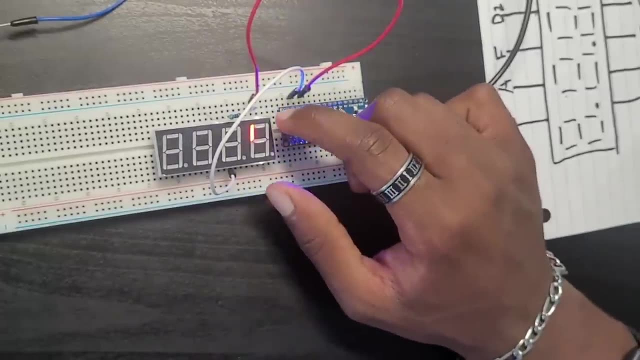 let me just say: okay, this lit up, so how do i extract the information right here? okay, this one, that is right here. okay, there's something right here. i'm just gonna again check it. it's the one at the very, very left. okay, i'm just gonna draw this diagram right here before. 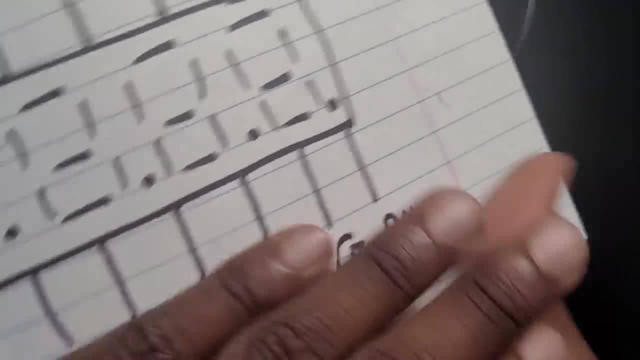 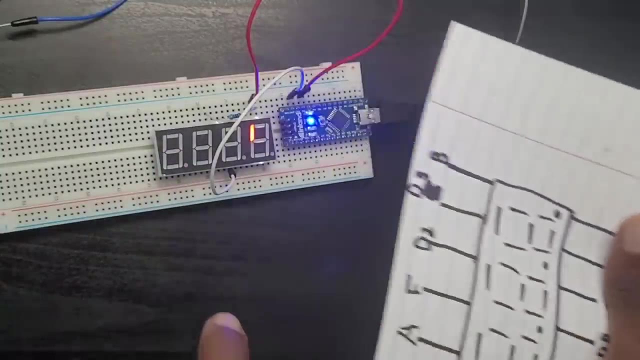 it. okay, let's just say i'm labeling it right now. okay, wait, let me just hide this one. i'll just hide this for now. there we go. let me just draw this diagram again. that looks like this and it shows the pins. so, right here, sliding up a what. it's lighting up at the what, at the fourth digit. 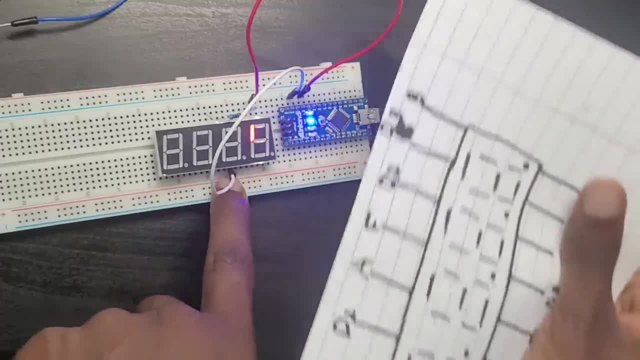 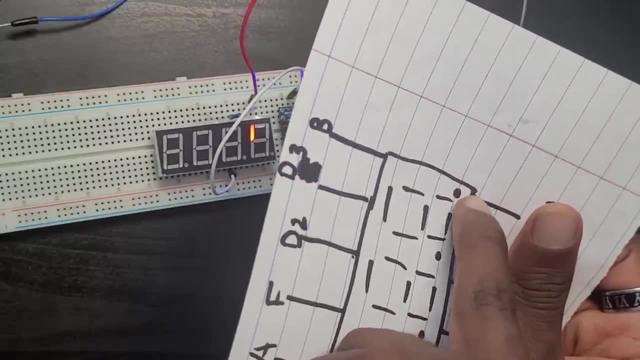 so what does this mean? this is the one that the very very, again at the very very right. so this one is supposed to be what this is supposed to be: digital. what, sorry? i said digital, i meant the digit number one. it's going to be digit number four. it's the fourth digit. 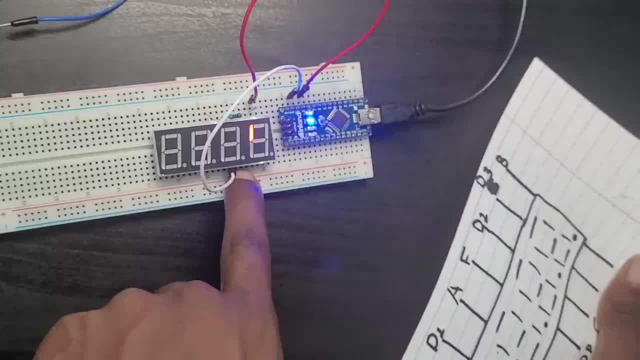 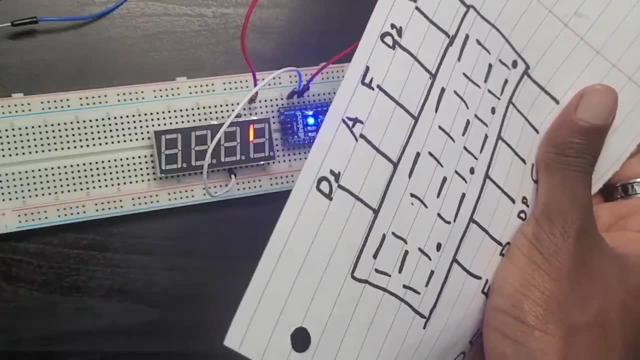 it's digit four. all right, so this is what this is going to be: d4. that is right. here it's going to be what i hooked it up to. here it's d4. what other information can we also extract? it's a common edit or a common cathode? it's a common cathode because why the d pins are what they're connected. 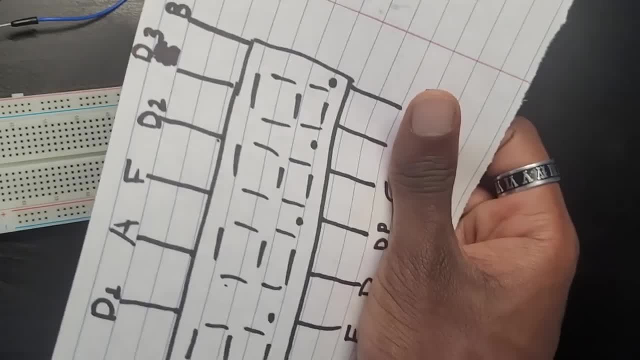 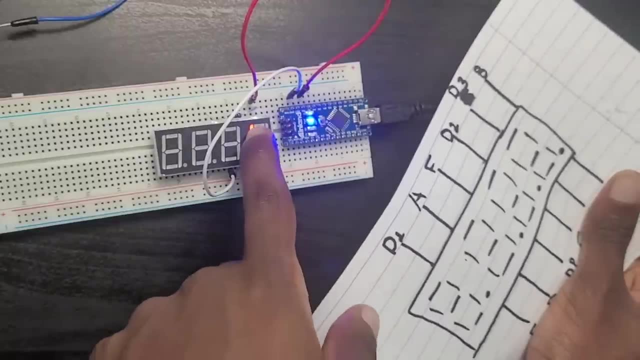 to what the gnd. okay, so they're what they're basically. what they're basically, uh, common, what common cathodes? okay, we extracted this information. what else can we extract here? can you see the segment right here? let me go over to my image right here, my screen, and 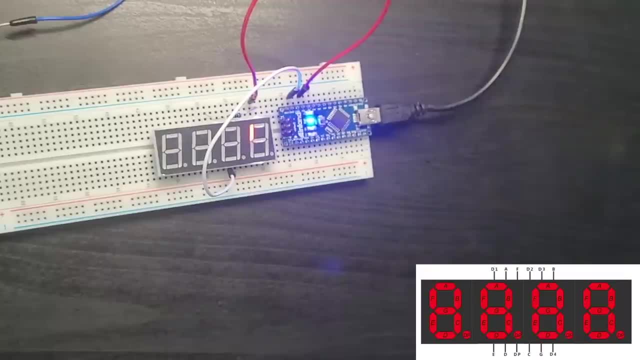 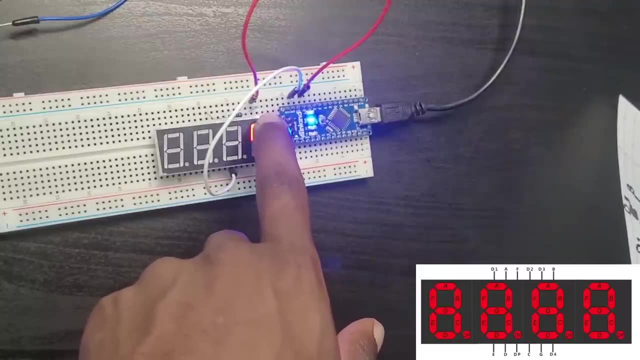 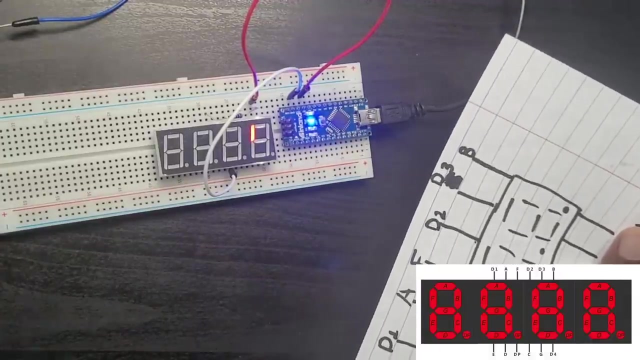 when you look right here, a is at the very top. so what does this mean? the segment be connected right here. okay, the segment be connected right here is what the segment be connected right here as well. it's going to be what it's: a. so this is what, if you, if you let's say, go here, let me just 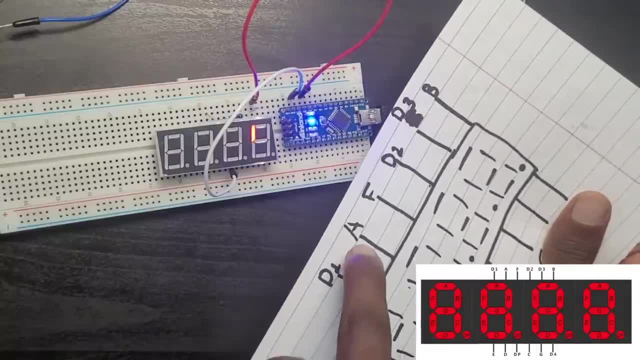 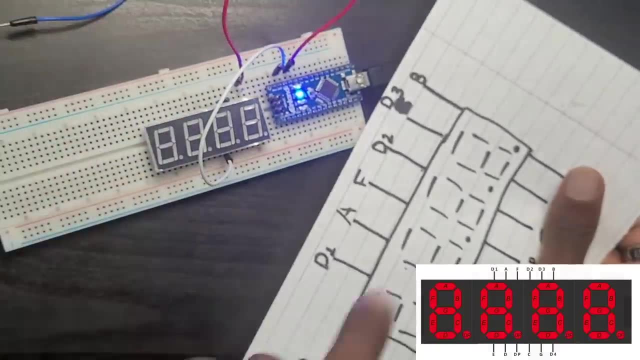 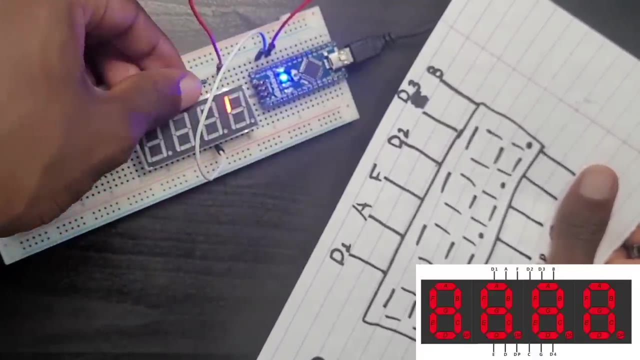 go over here. there we go. the one that we connected right here is a. when you look at the resistance right here, the leg of the resistance is touching a. can you see it? it's touching a. there we go a. oh, i just moved the resistance again. that's the resistance, that's uh. oh, there we go. i moved the. 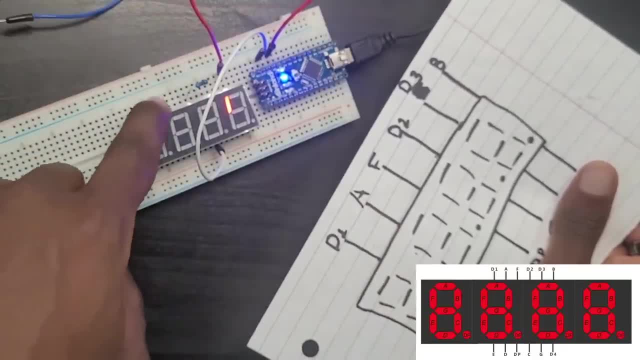 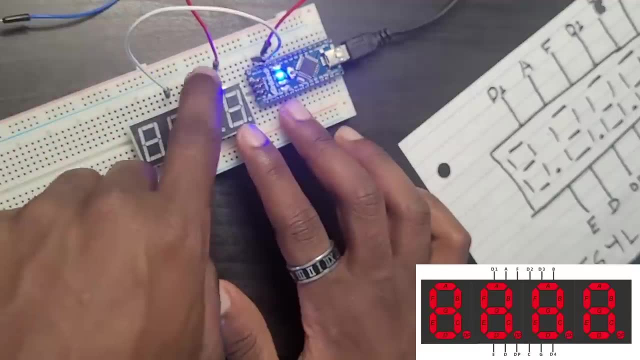 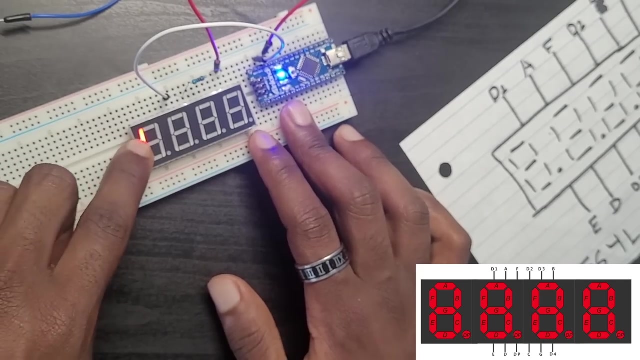 resistance. there we go a. so i also discovered a pin right here. additional pin, let me just go over to it. hmm, it's around here, i think. so it's around here. there we go now. what is this? this is what. now we can just again look where it's located right here. 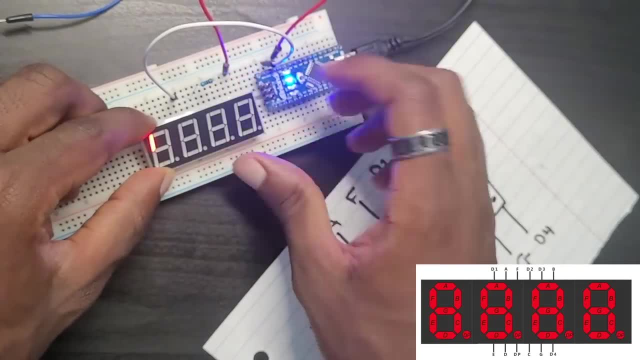 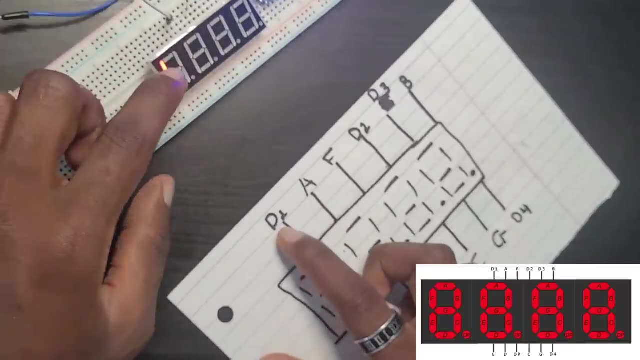 what will? we connect it right here and then we can say: what is this again? let me just move this to the top. can we see it? it's the one at the very, very, what? at the very edge? what is this then? it's appearing on digit one. so basically it's what, it's d1 right here, when it. 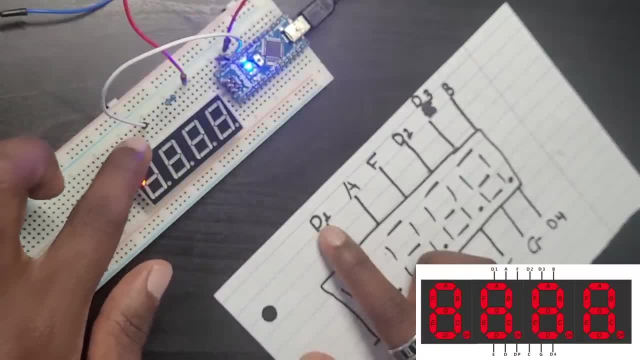 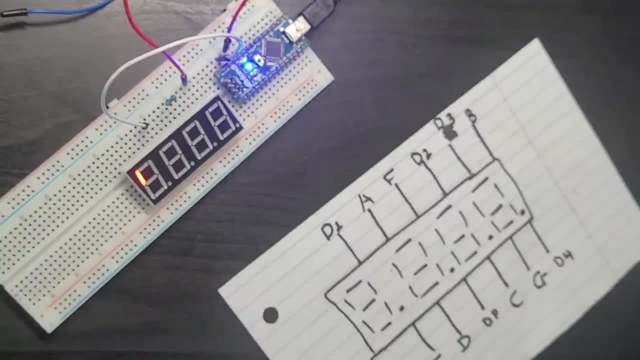 comes to white one again, the white um wire slick. it's going to be connected to what? the d1? okay, what is this again? a. so we can keep finding them again. by doing what? by lighting up other segments. that's all you need to do. so let's say we're trying to find another segment. what do we do? 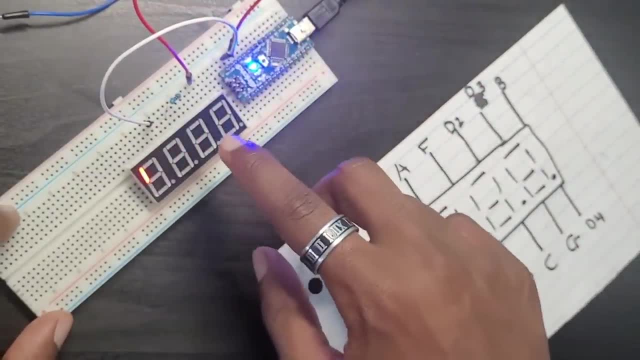 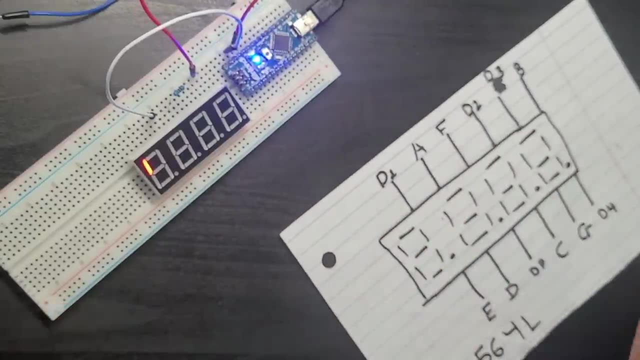 right here. we're going to move our resistance right here. and what does when it does not light up? what does it mean when it does not light up? it's part? it's probably what. it's probably a what a d pin. so we're not going to touch that, so we're going to leave it again. we're going to light up all the. 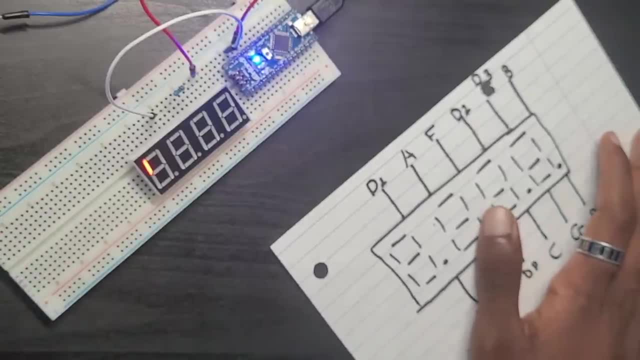 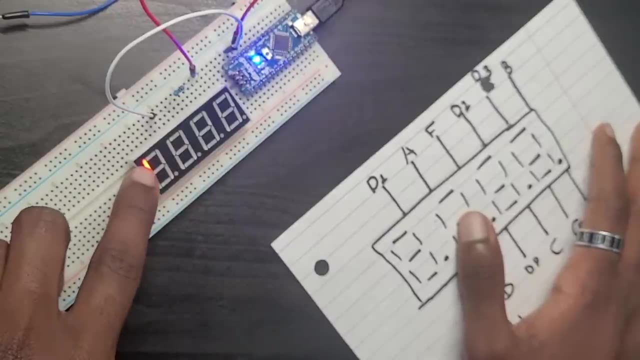 segments. so basically, let's just trial and error until you find one segment. as soon as you find, as soon as one segment lights up, you can extract lots of information from here. i can extract what this is a- okay, this is a. from here, from the red wire, i can say this: 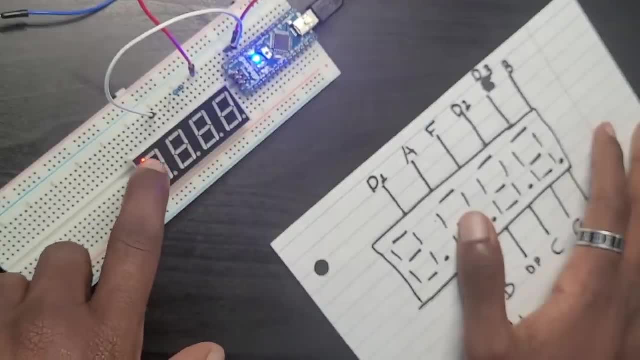 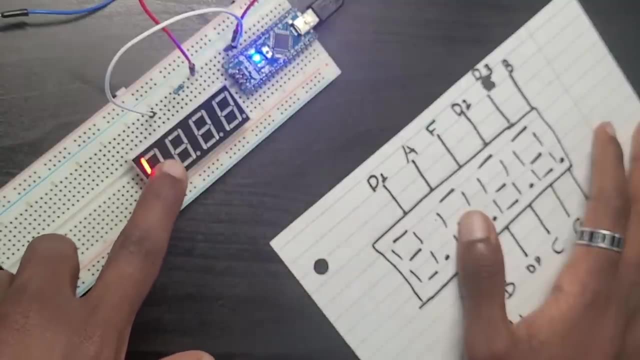 the pin. right here is a. what else is it? it's on the first digit. so it's what? so it's going to be what the digit number one is going to be here. what else can i extract? right here i can say it's a common anode or a common cathode. so again, you keep doing that and find. 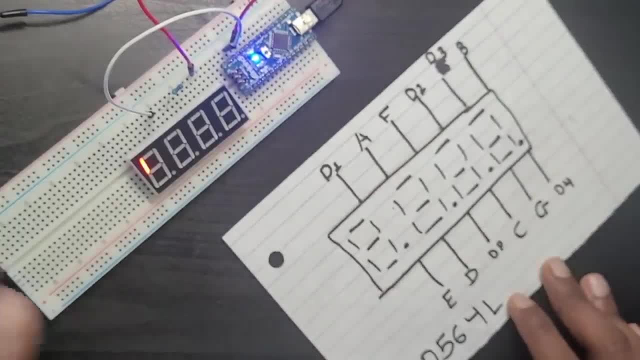 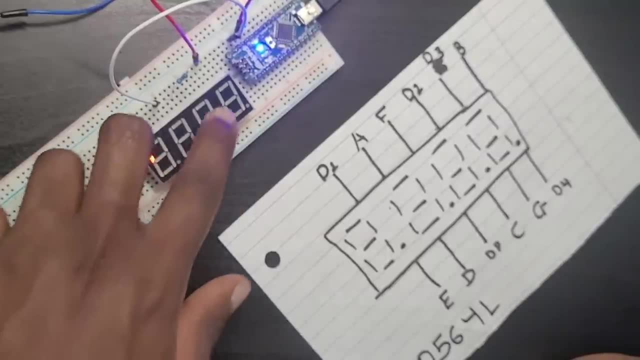 all the pins, okay, and name all of them. that's all you need to do. so, with that in mind, we're going to actually work on a project in the next section and we're actually going to wire up all of this, which is going to be a lot of it. so we're going to wire up 12.. so, anyways, we're going to 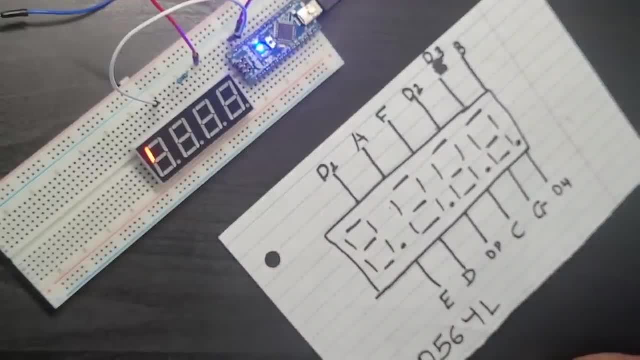 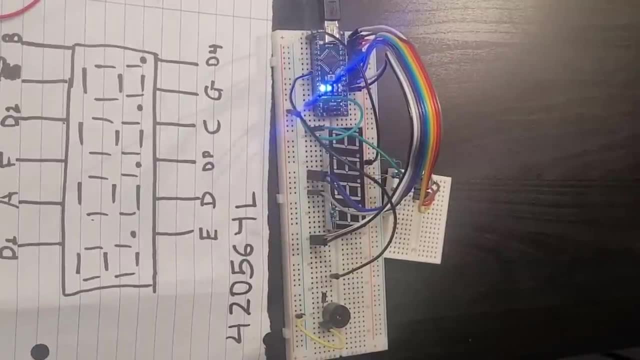 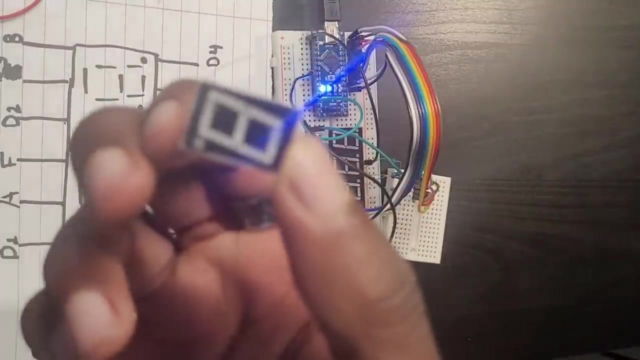 see you and see you in the next section. we're actually going to work on a project with this one, okay. so we're going to build as a timer, okay. it's like how we did using the one segment led display right here, one, the seven segment led display with the one that has one digit. it's. 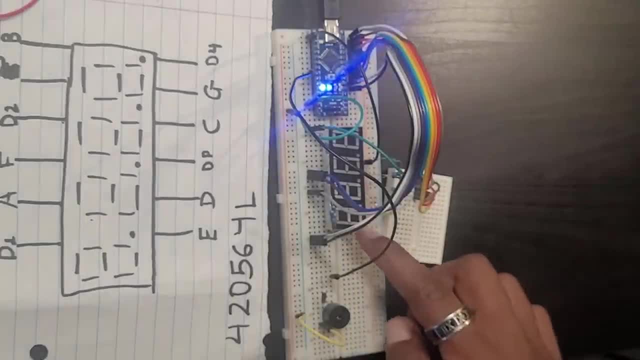 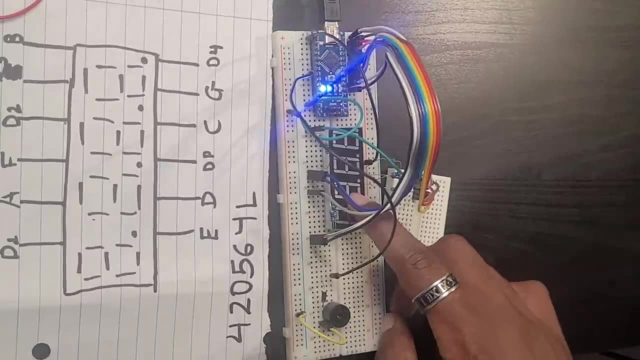 like how we did that. we're going to be building a timer and it's also going to be including a buzzer. okay, it's going to have a buzzer right here, an active buzzer, and it's going to actually ring after what the timer hits zero, okay. so just to save you guys time, i did all the 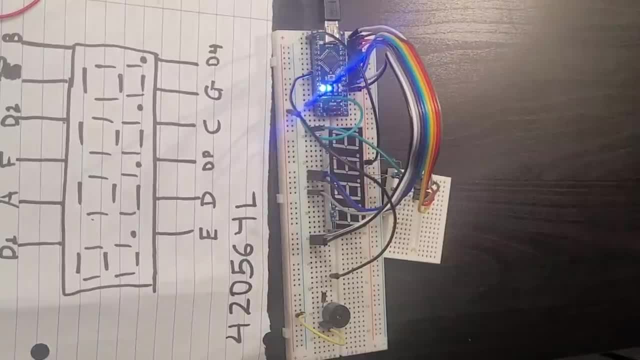 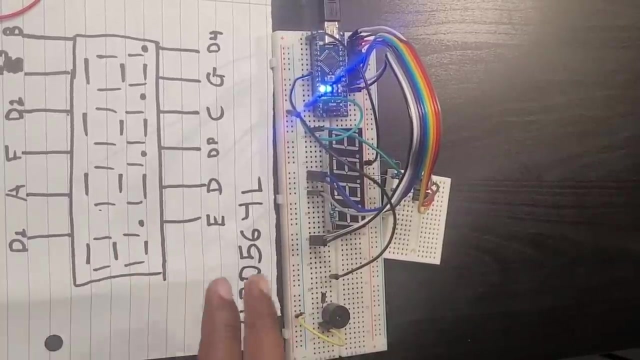 wiring up that was necessary again. so i did every wiring up and threw down all of the all of them as variables. so let me just again get this closer so you can have a good look at it and what, which, where, where it's going. so let me just make a simple again. let me just explain it simply. 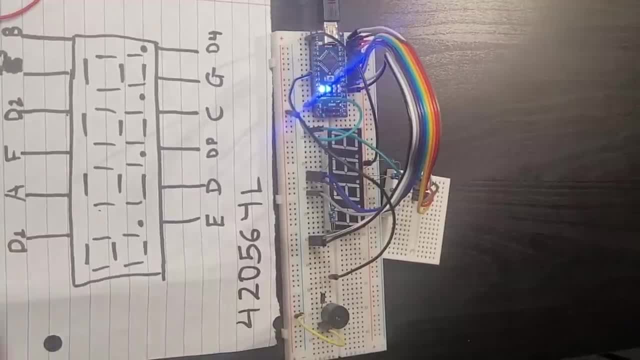 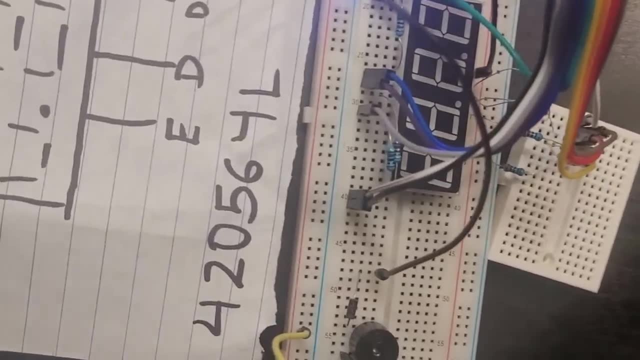 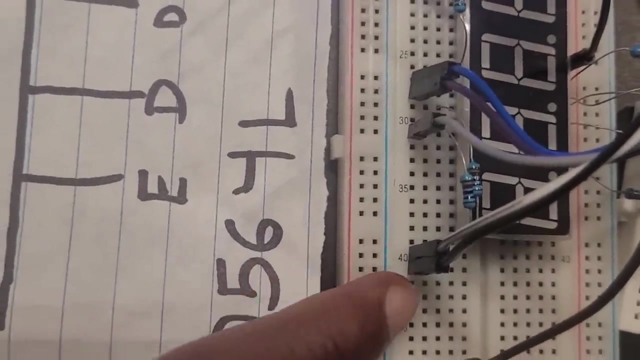 these are a and f, the. let me just again bring this closer. how am i supposed to do that? let me, it's actually hard. let me just bring the camera down. this time it makes more sense to do that. there we go. let me just bring it way closer here. all right, so these two, as you can see, the black. 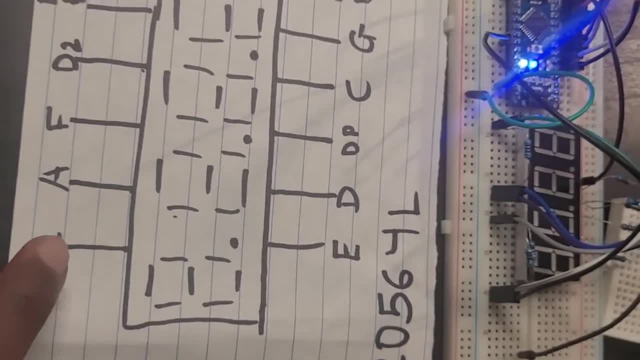 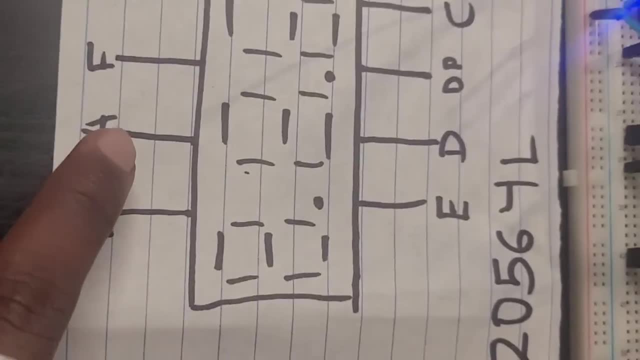 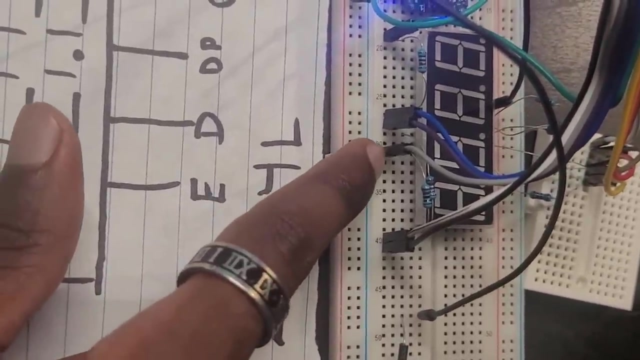 and the silver. again, when you look at them, they're connected to what? to a and f. they're connected to resistors, right here, one resistor leading to a and the second resistor leading to what, leading to f. okay, that's all i did. then afterwards, what i did was okay. what i did was i put this again as you. 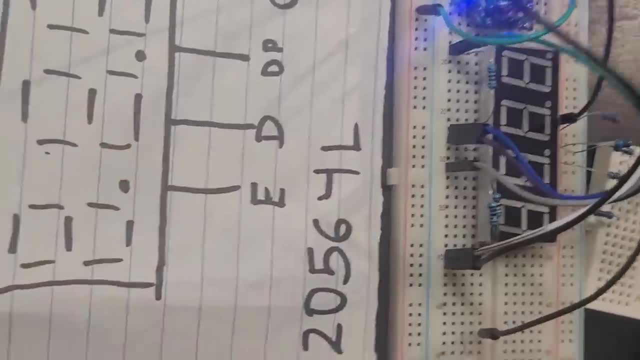 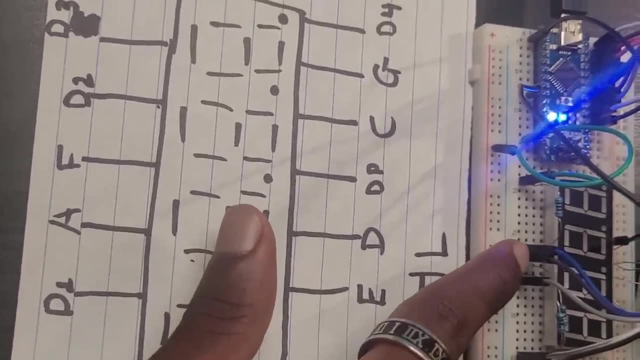 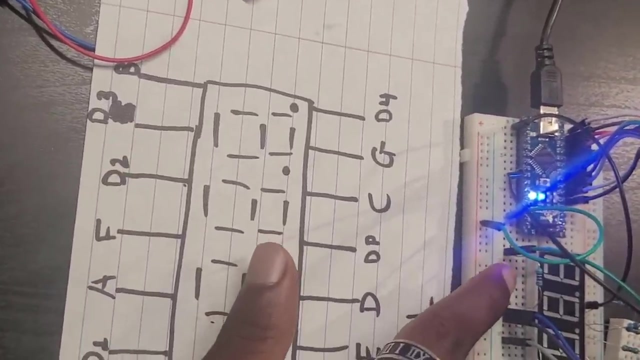 can see right, right here. can you see this? the silver one. the silver one is supposed to be d1. okay, it's d1. and afterwards these two colors right here, the purple and the blue respectively, are d2 and d3. and finally, i set a resistor for again b, because it's a segment again. 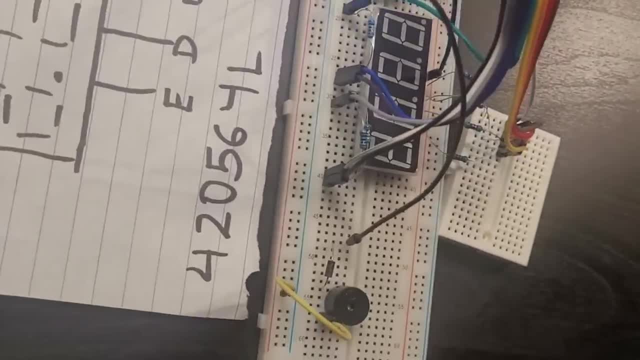 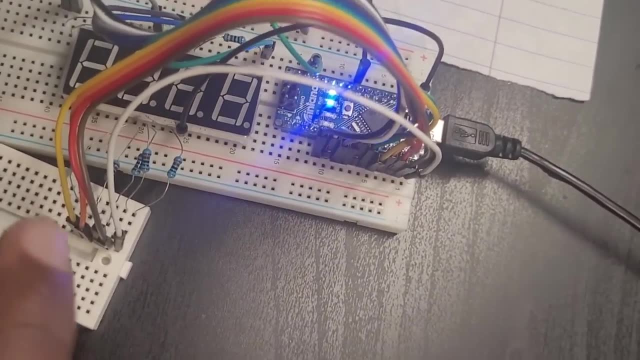 and then use the green color. okay, then afterwards, what i did was: okay, i went to the other side because i did not have space in this side too. as you can see, i don't have space on this side, so i just used another small breadboard just to go through it, just like how i did using the one. 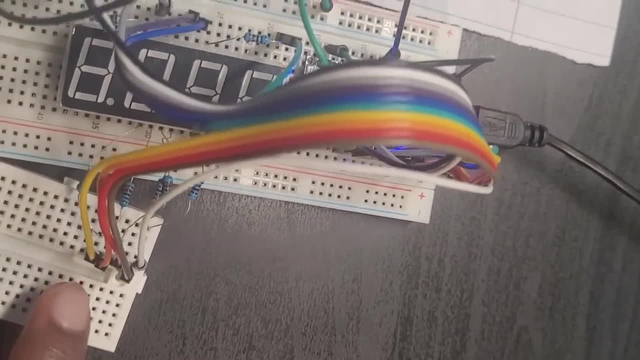 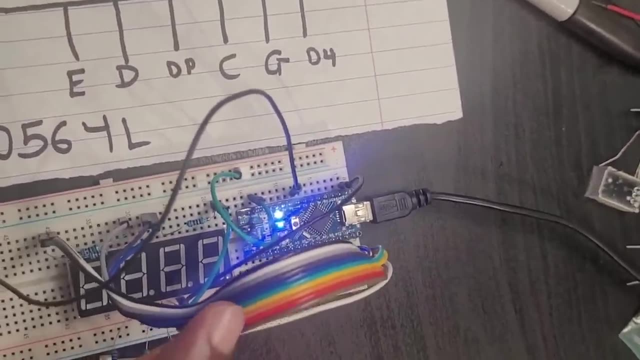 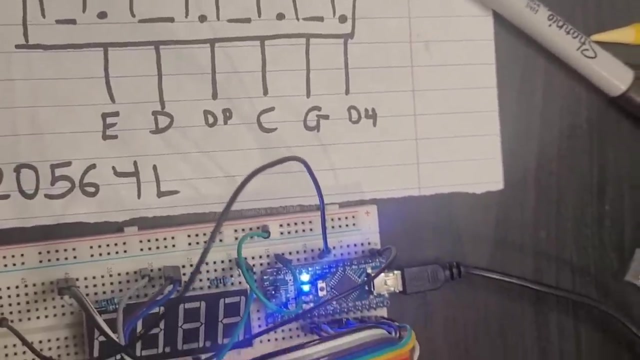 which is seven segment led display. so what i did was again connect again these pins, again these pins, in order. right here we start from yellow again. the next color is yellow, as you can see on the stripe- and then connected them respectively. so yellow represents e, then orange represents d, obviously, then red represents dp and then the brown represents c. 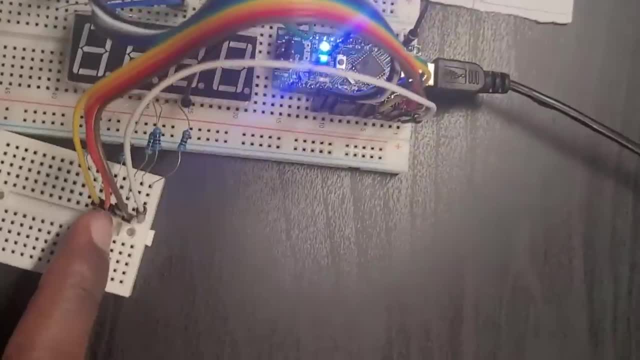 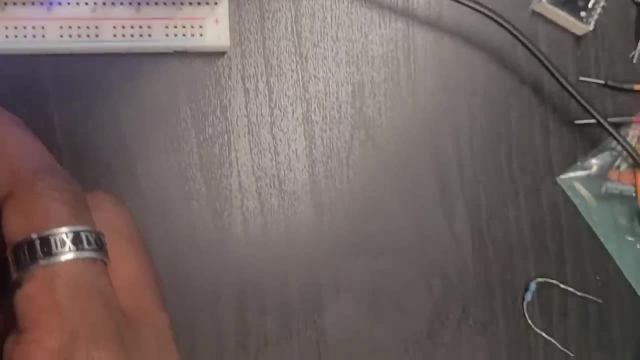 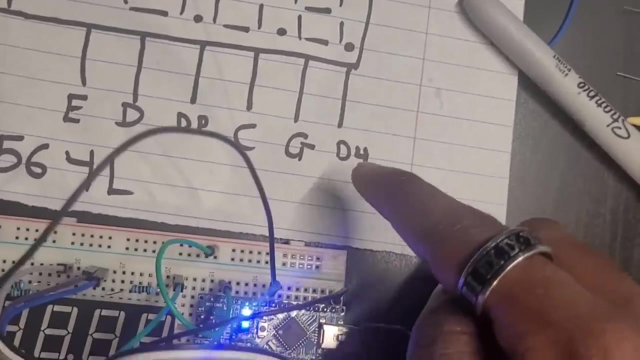 and then, right here, because i run out of wires, right here again, we're connecting lots of pins because i run out of wires, what i did was used a single white wire right here, specifically a single- what white wire right here, as you can see it, and this is connected to what is connected to g. okay, and one final thing is obviously we 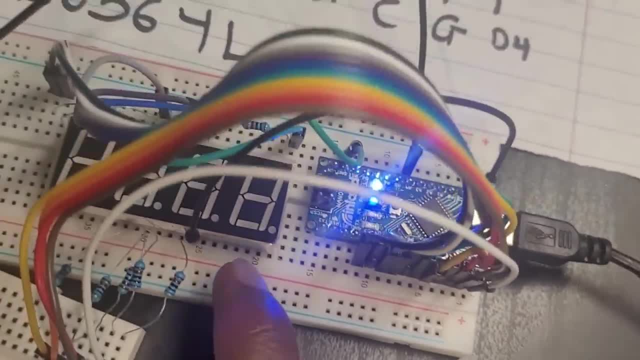 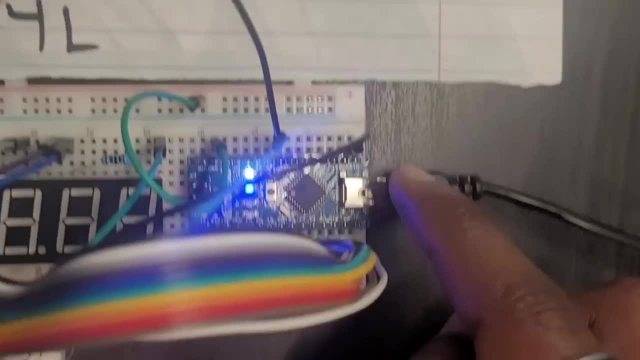 have d4 right here that i'm going to use. let me go back right here. obviously, i don't have to put a resistor on this, so i put it right here and connected it to what? pin 13. okay, can you see? pin 13 is at the very, very other side. let me just again just give this. let me change the color. 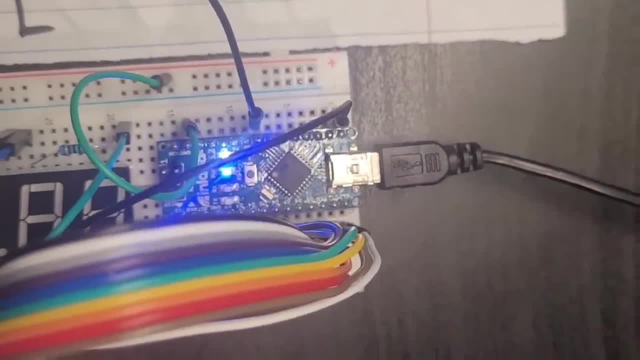 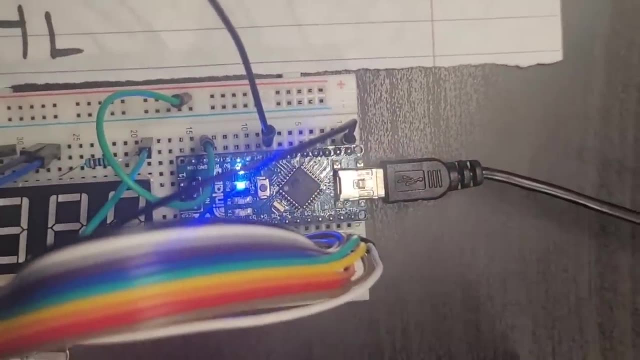 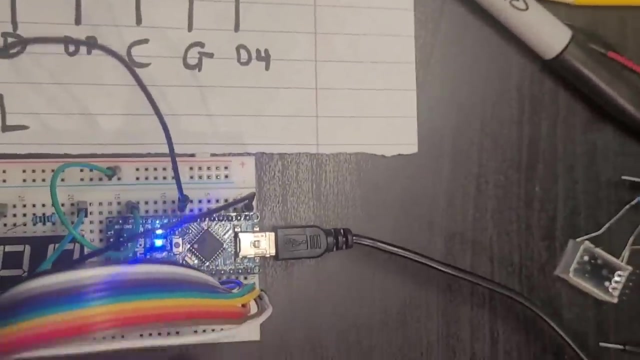 so better change it to: there we go. this is better. there we go, d13. all right, d13 is right here. the distal pin- what 13? again, you can see it from another angle. there we go, distal pin 13. so that's what i did: i connected them and separately, i run out of distal pins, right here, okay. so one thing: i 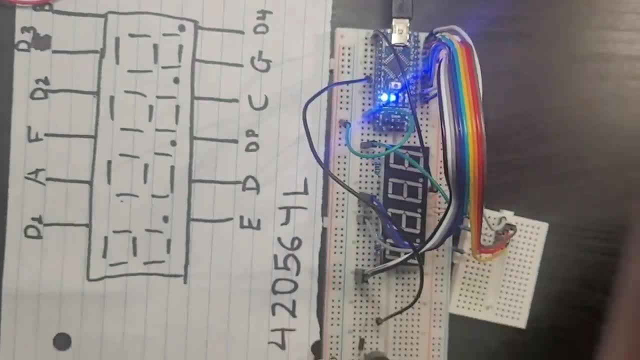 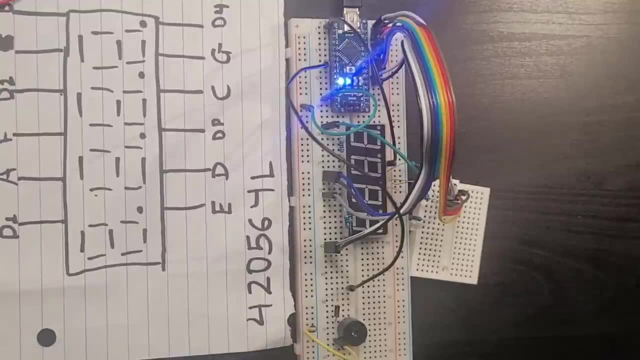 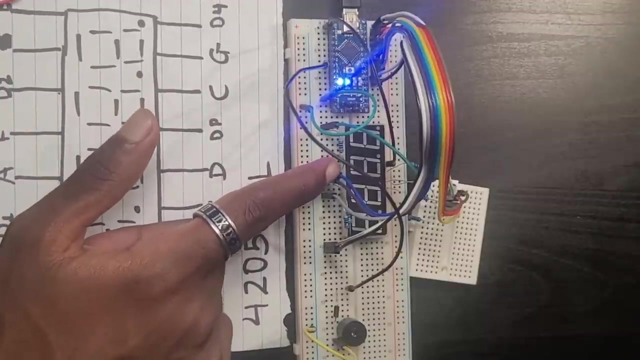 want you to keep in mind. let me just put this in its normal angle. okay, there we go. so one thing i did right here is what, after i was done with setting up the four led, again four digit led, matrix led, uh, segments right here, what i did was what? i set up a different circuit, a big black one. 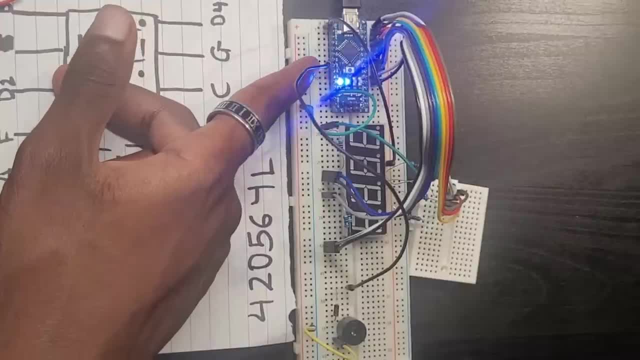 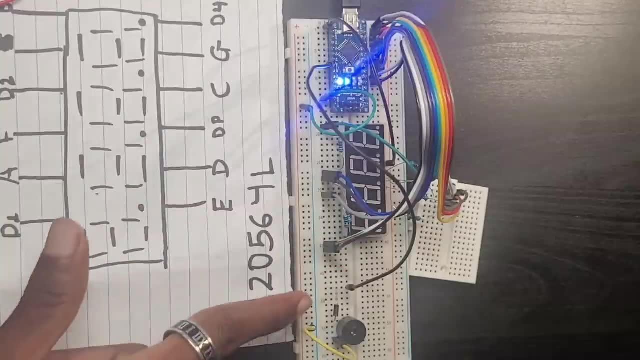 i used an analog pin because i ran out of a digital pin right here. i used an analog pin. okay, i used what i used, an analog pin. and then i used a diode. okay, a diode again, as i said, supposed to change what it's supposed to change: ac. 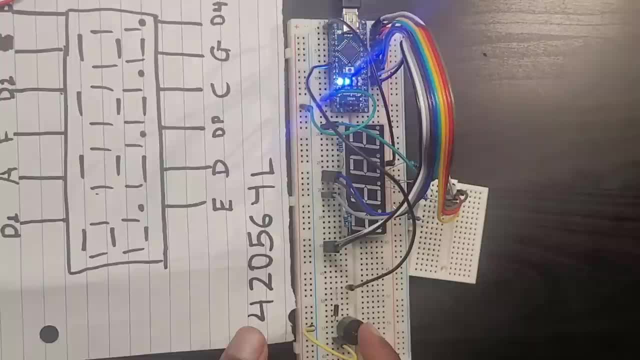 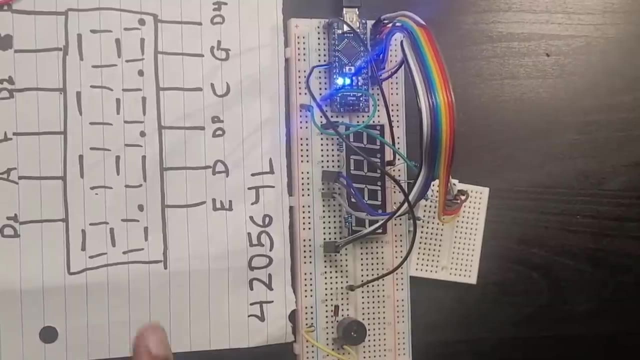 to dc circuit. all right, and then i used my active buzzer. active buzzer, as i always told you guys, it it's what it needs: five volt dc. it receives what? five volt dc direct current and basically, what again? what does? uh, let me just explain the science before we go behind it. uh, what does the diode do? 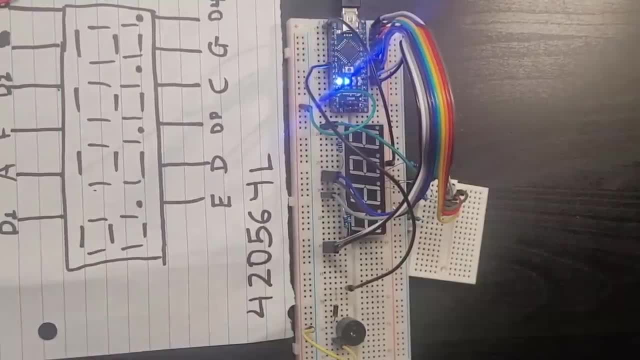 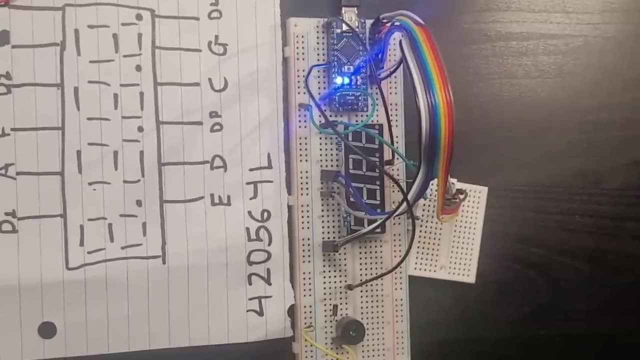 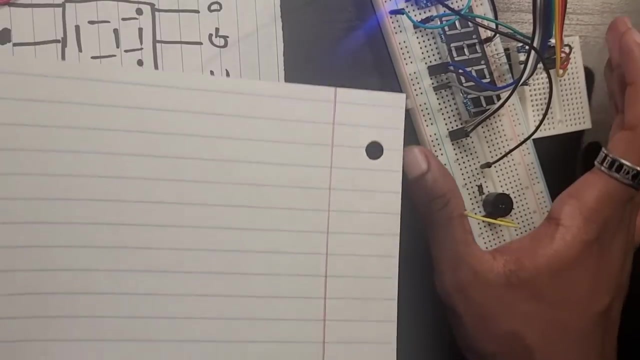 it basically can convert ac to dc. let me just show you how it does. let me just bring the paper right here. let's go before. you know we keep walking and focus on the again, this, the four digit, uh, the four digit, this four digit display, because it's going to be the main one right here, it's the main component here. 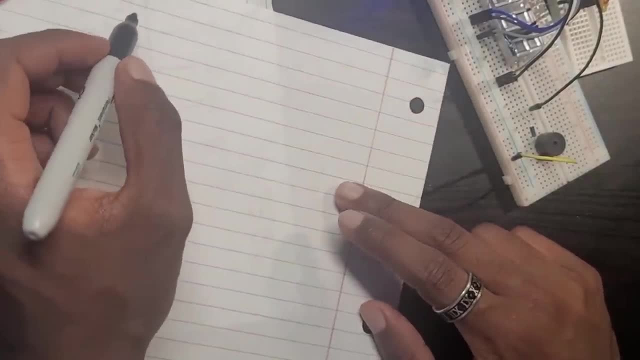 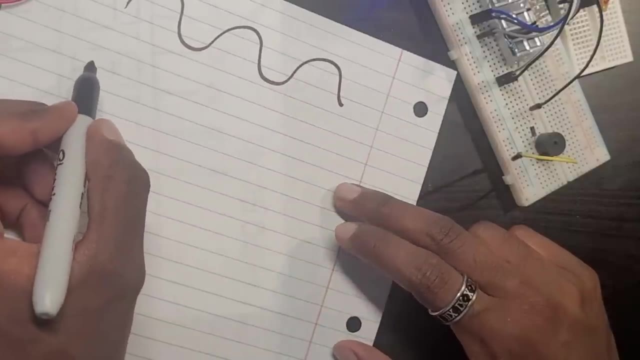 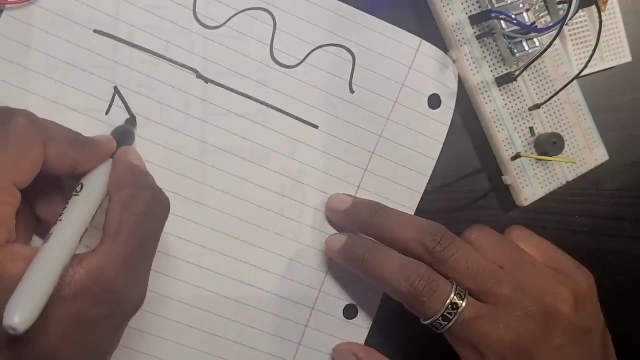 basically, when we use a diode, if you remember, ac circuit goes both sides. it goes both sides. okay. when it comes to dc circuit, it only goes. what one way? okay, it's straight, it goes one way. when it comes to a diode, if you remember, i told you guys, even when we're using this led, it's going to go. 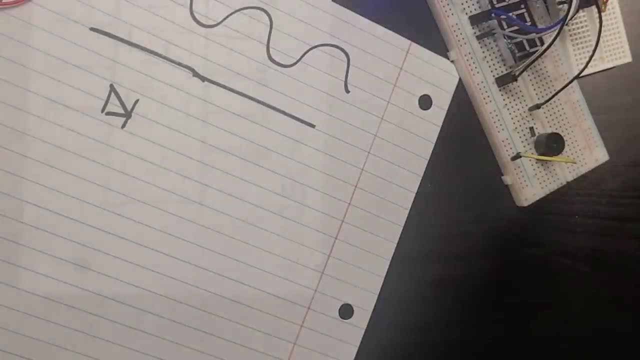 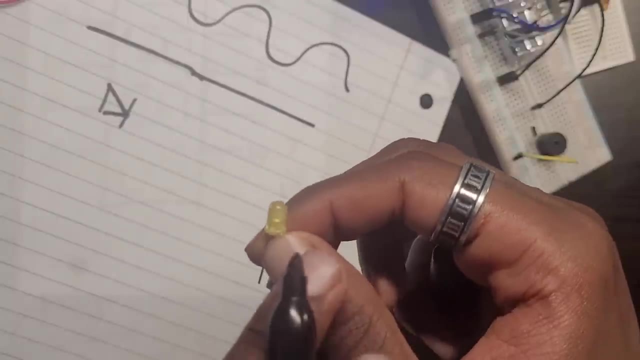 both ways these. let's bring an led right here. i think an led would be a great example, because they're diode's too. they're literally what light emitting diode's. they're diode's, but they what they emit light. that's their like special property, but they're just diodes. they're the same thing. 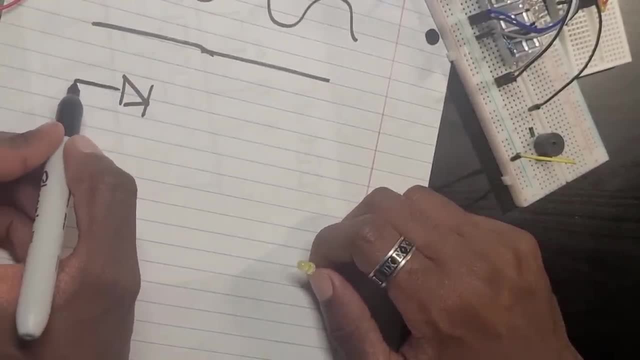 okay. so when it came towards um, these again diodes. they represent like this, if you remember, and then we again presented them in the circuit. so this is what the positive side and this was what the negative side. okay, is it the positive and the negative? i think i actually changed it. 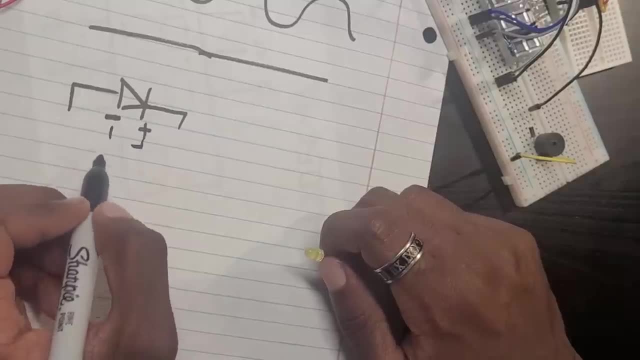 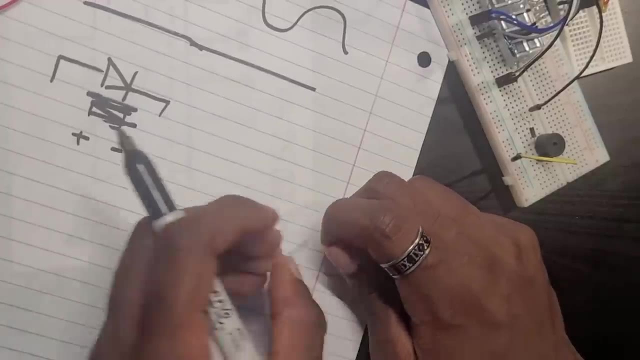 because now we have additionalurger also right here. so these are theикi, theics again. these are actually switched it up. there we go. it's this side, it's positive and negative here. anyways, the main thing here is what the main thing here is: if we connect it to the positive again, we connect the 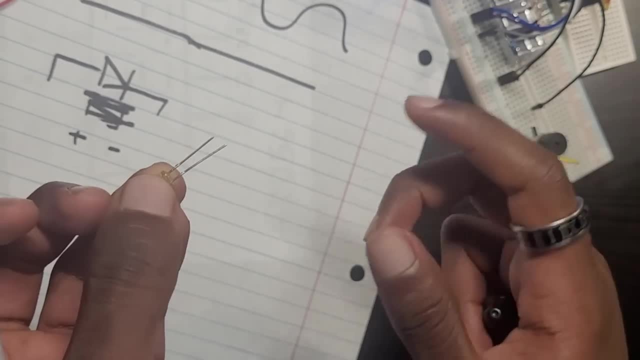 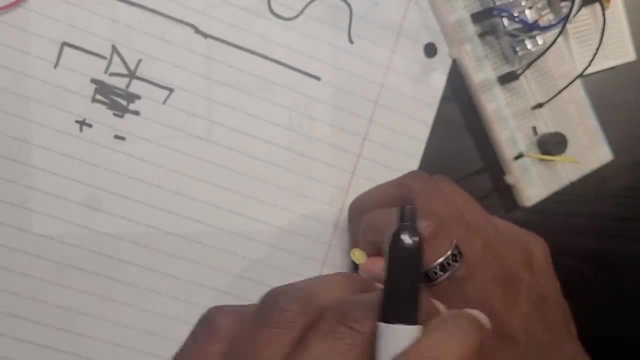 positive to the 5 volt and the negative to the gnd. it worked. but if we switch the direction, what happened? it did not work. so, basically, what happens in diodes? in diodes, currents only flow in what. currents only flow in one direction. as i told you guys, currents only flow in what? 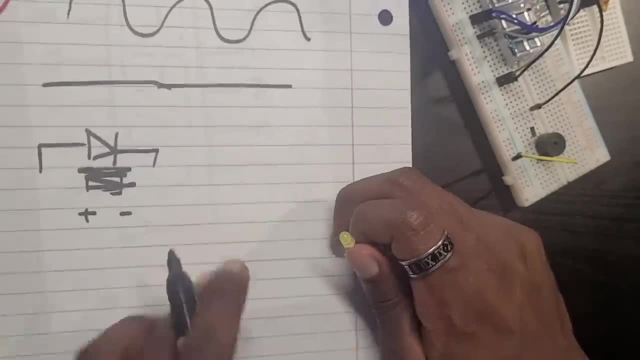 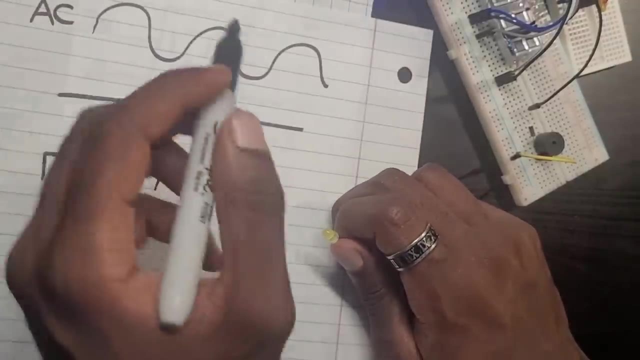 in only one direction. so that's basically what it's doing. when we receive again inputs from analog pins and digital pins, they're always what? as i said again, they're always ac. so to just change it to 5 volt dc, what does the diode do? diode only receives what half of what the ac is sending it's. 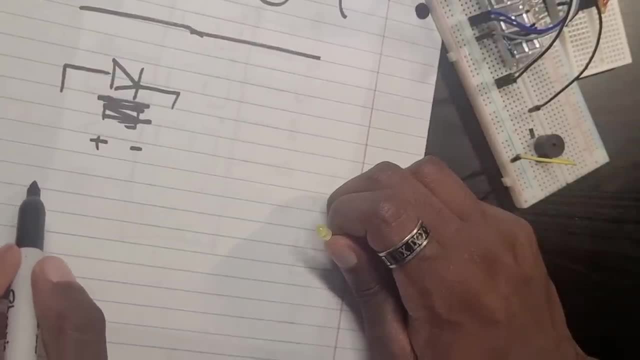 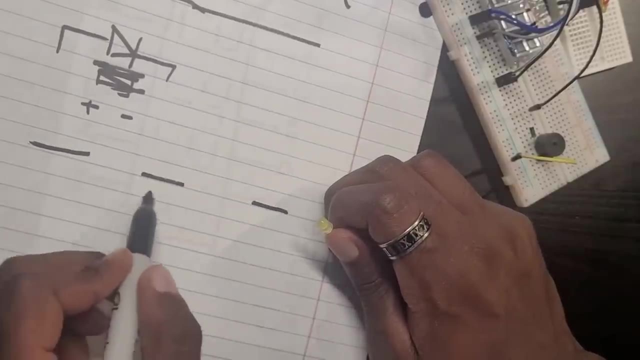 going to be receiving half of it. so basically it's going in both directions. it's going to receive only the one direction and it's going to what it's not going to receive the other one. it's going to be dull and then keep on doing this. so basically, over time it looks something like this: if you just 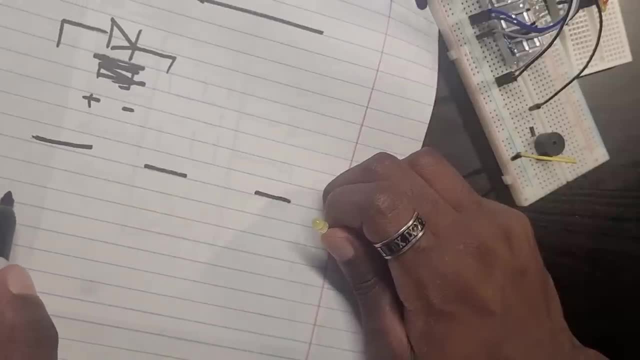 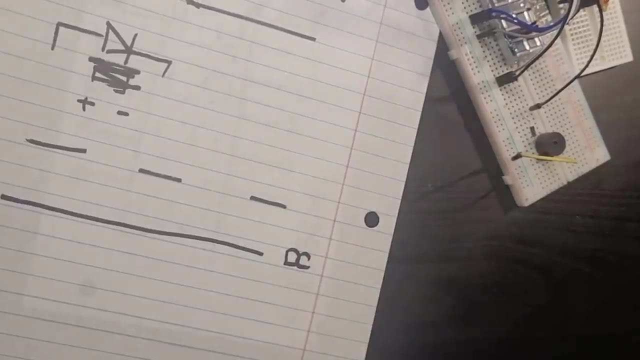 again lower it down. let's just say, we tune it down. it's going to be almost as if we're getting what we're getting: dc circuit. okay, this is just as if we're getting dc circuit. that's one thing i want you guys to keep in mind, okay, when we're working with this a diode. let me just show you guys what. 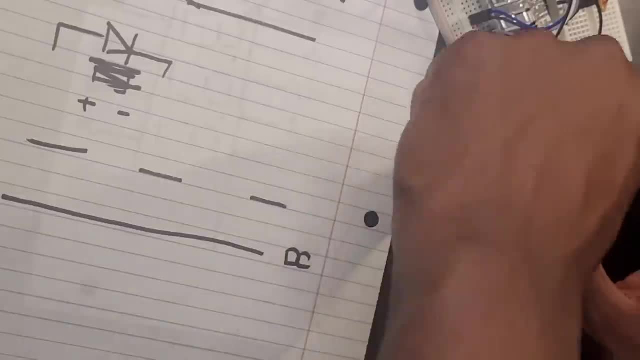 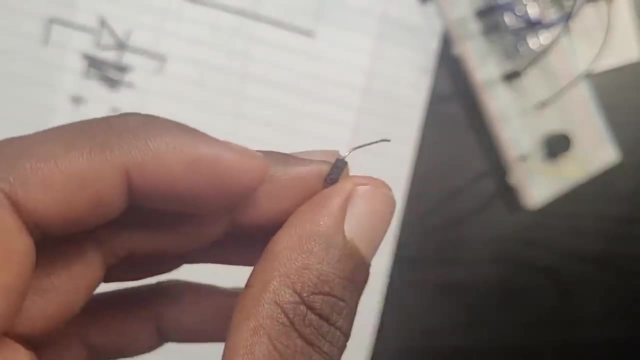 a diode looks like this is called a rectifier diode. again, read your labels and try to find some sort of diode. okay, this is a rectifier diode, right here. okay, basically, does what changes what it's used for what? basically, to change ac circuit to what to. 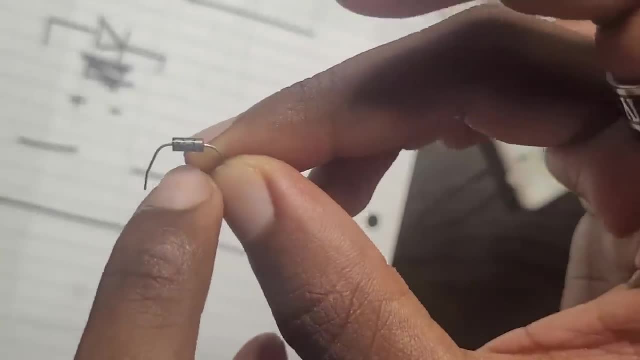 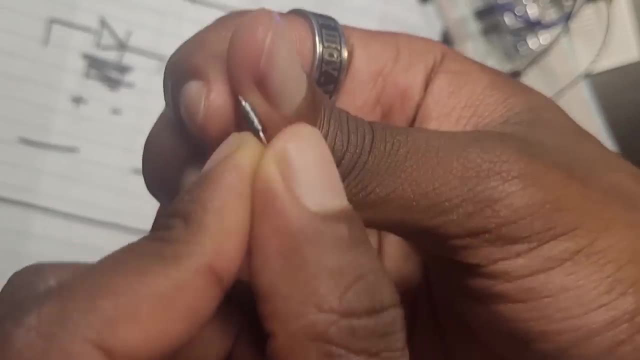 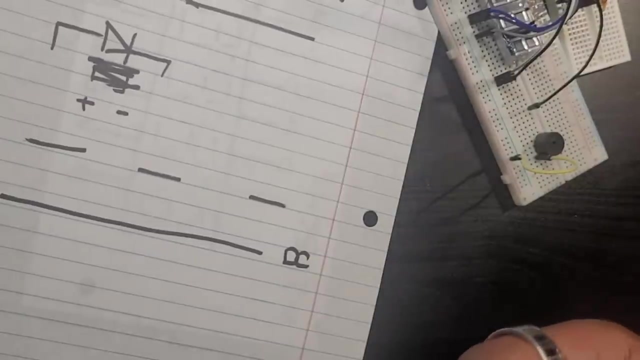 dc circuit. okay, again the side. again you have to understand the side. okay, how you set it up is again important because the diode, if i just again change the direction right here and put it like this: if i put the there we go. if i put the again silver mark right here with the, with the positive, 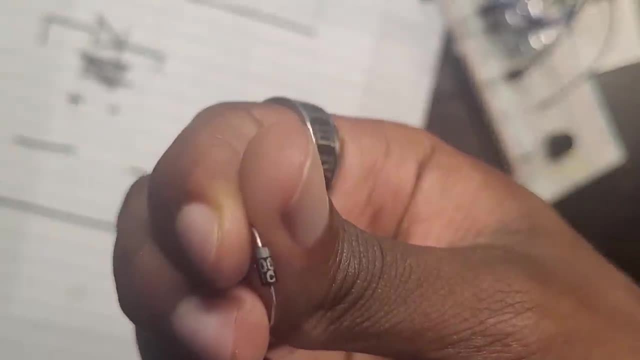 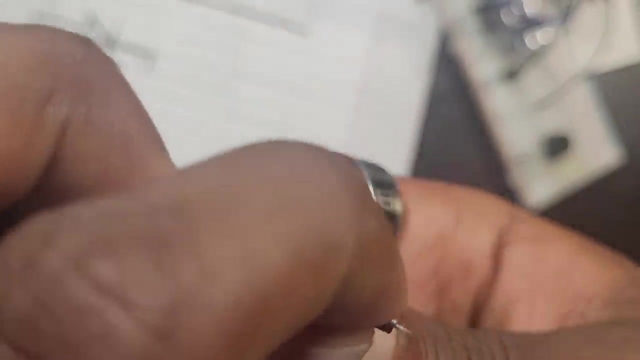 sign. okay, with the positive sign, what's going to happen is what it's going to basically, what it's not going to connect. it's basically going to be silent. but if i obviously change the direction right now, i change the direction. it's supposed to be like this. if i change the direction, like 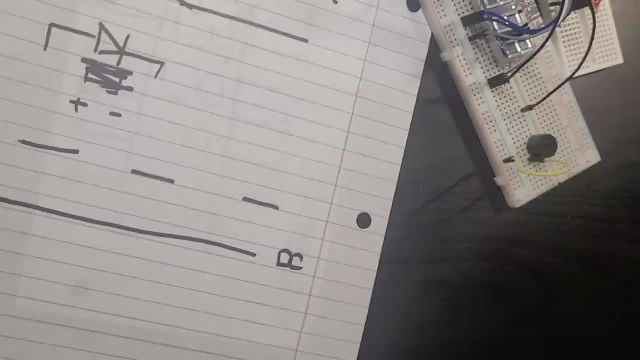 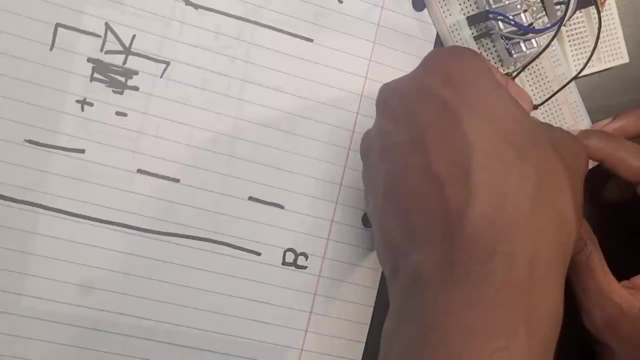 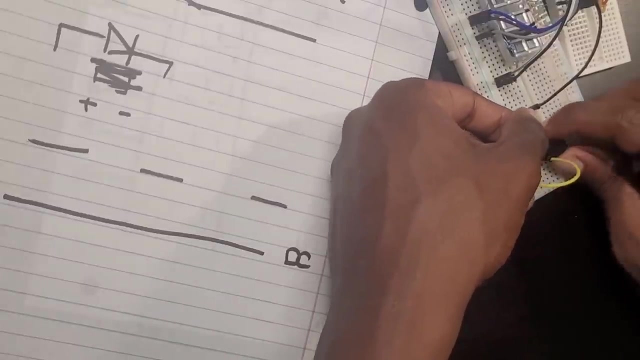 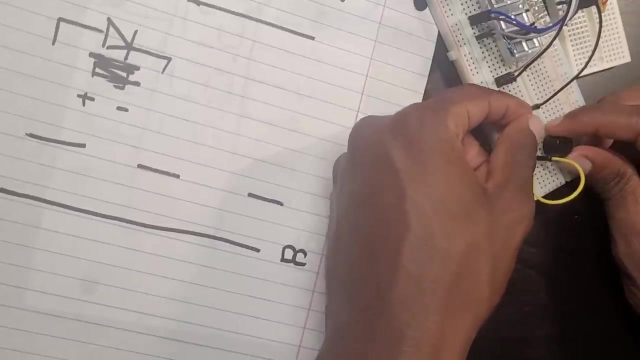 this, it's going to work perfectly fine. okay, just keep that in mind. let me just put it back to its spot, though. go one, two, ruin, ruin it. oh, i think i bended it a bit. i don't think it's on the positive side of the. okay, there we go. the positives here, all right, there we go. connected it, obviously, if 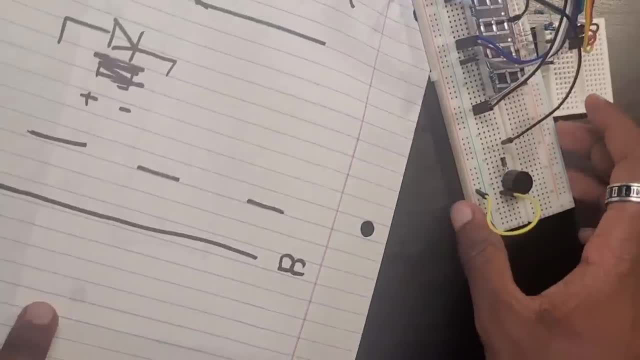 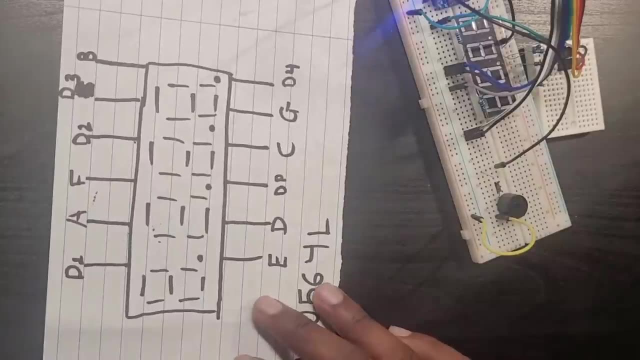 i don't hear anything. i just set it up wrong again. we can know that it's not going to work from just again listening to it. if you don't receive anything, then basically what i did is what. what i did is change the direction. okay, let me get this out of the way and the gnd, if you can. 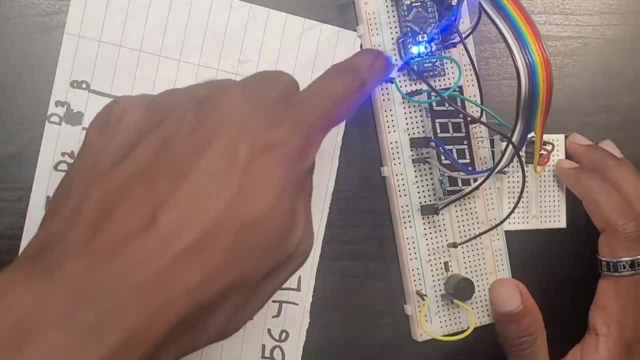 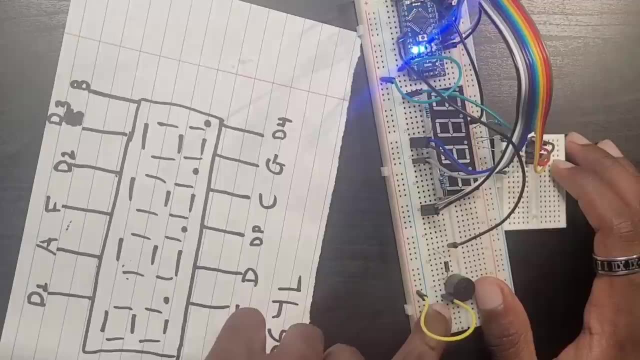 see right here the gnd. let me just make sure you can see it. the gnd is again extended by this. it goes the whole way here and then what happens? it goes what? to this side and then it goes to the other side of the what, the active buzzer. okay, so now let's focus back on the again fourth segment. 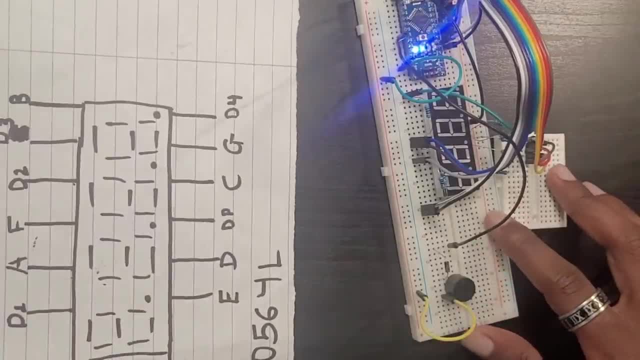 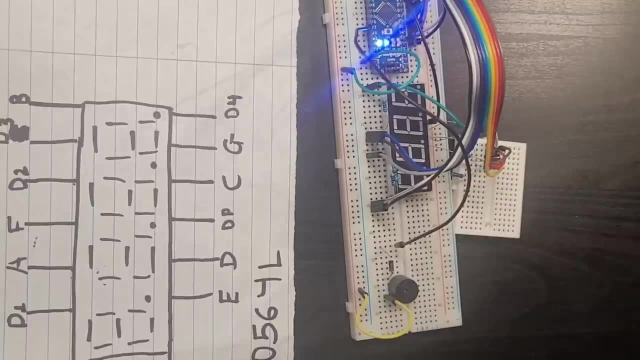 led display. so everything before obviously we start with you want to do is what we want to check if everything's hooked up properly, especially the resistors. again, there might be cases where, again, the resistors are not connected properly. basically, i have to push them in, so let's just see if they're connected properly. so let me go. 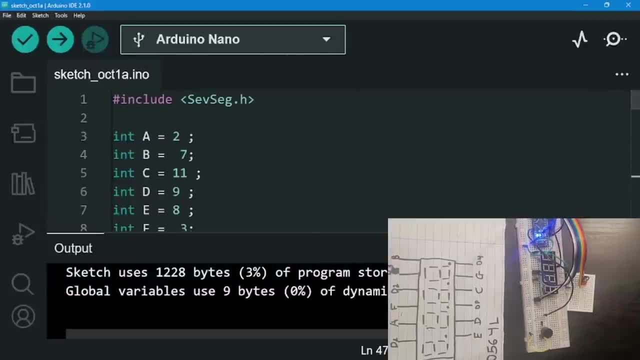 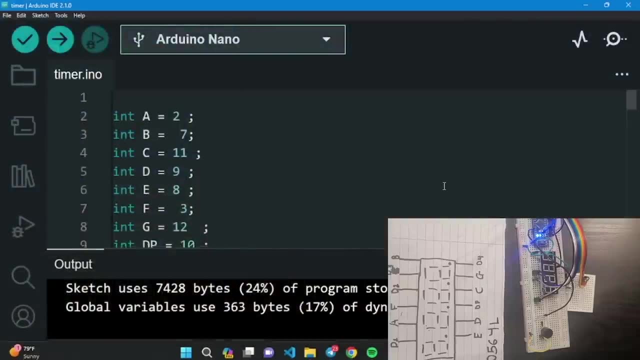 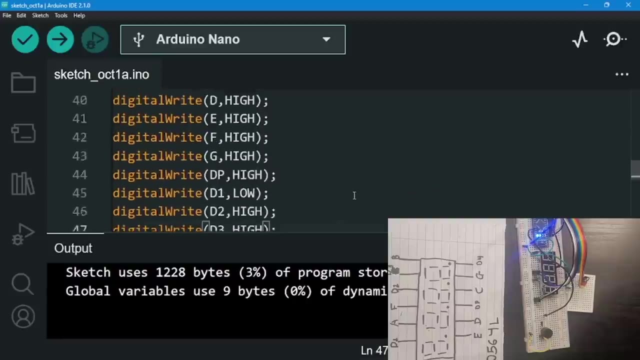 over here to my code. let me just do that. i have another code. i want not this one, i think it's this one. no, it's definitely not this one. how about this one? i think it's this one. there we go. okay, let me just remove this code. i don't need this. i'm going to go back to this. 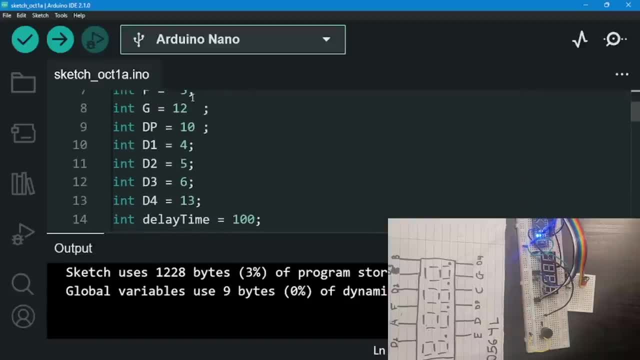 we're going to be including libraries, so we're going to get back to this, but we want to do is check everything. so, again, i just set up the pins again, give them the name and then connected them to their what to their again the pins that, um, we had to use. again to the respective pins, uh, one. 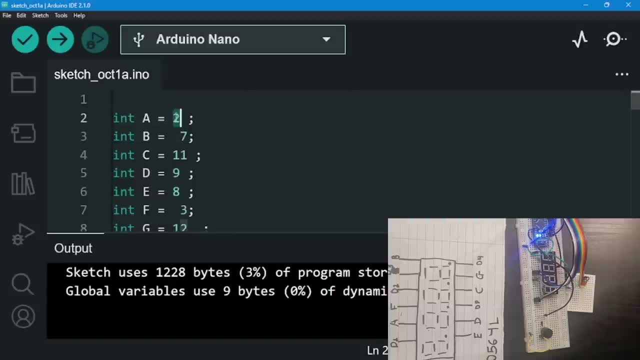 thing you notice here is: i again recommend that you don't use digital pin one and pin two, because again, they're used for what? for binary. but this time i was using digital pin one. why is that? so you can see, i did not have any space. i finished one until 13.. i used every pin until 13.. and we 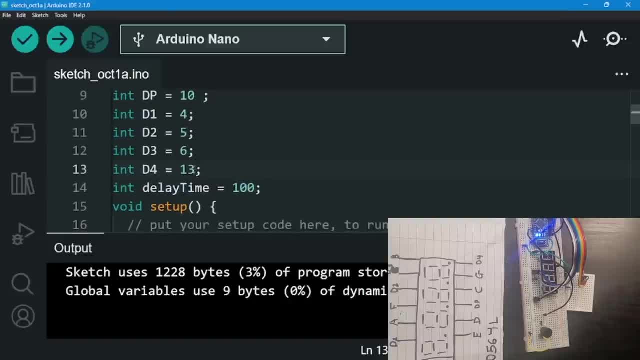 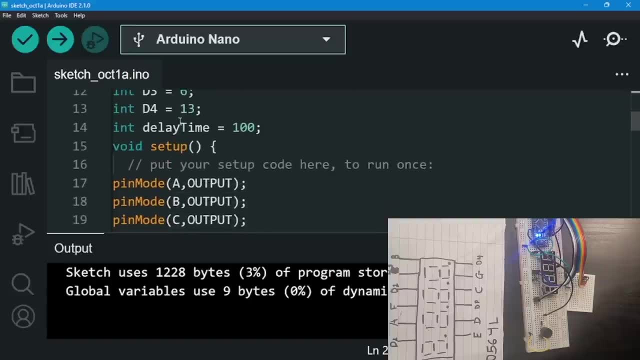 have up to 13, and i used every digital pin that i had, okay, so that's why i used two. again, you can use them, but most cases when you don't need to, don't use them, okay. so again, we're going to start here and then again i set up everything- d1, d2, d3, d4- and then i set up a delay time, set it to 100. 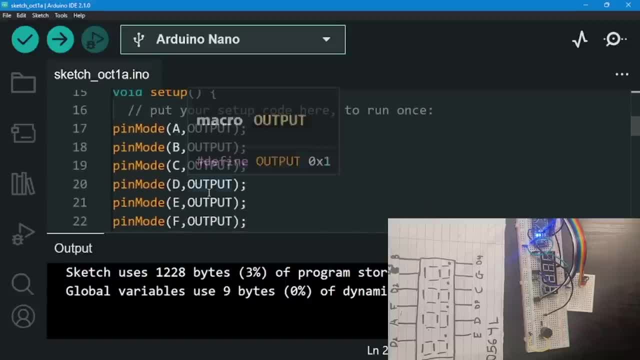 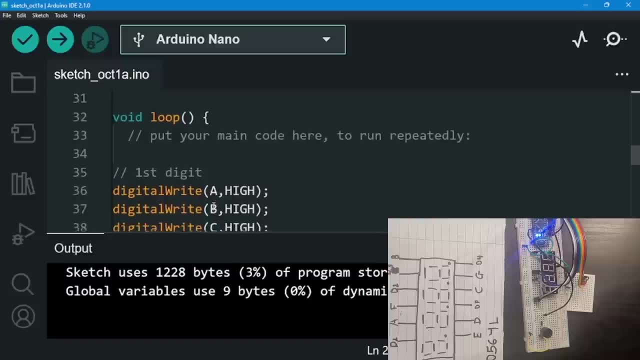 milliseconds we're going to get to it. and then obviously i have to set everything to a ton output, which is like how we did in the in the one digit seven segment led display. just did the exactly same thing and i set every segment to high so we can see it, including the decimal point, and then 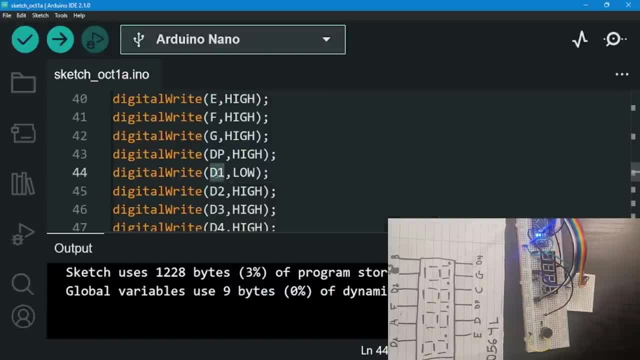 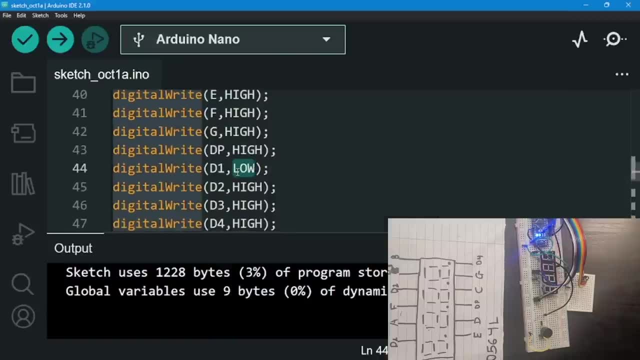 obviously, what do we do? we're going to again using a common cathode. so in this case, we want the gnd, so the one we want to light up right now. we're going to set it to what as a gnd. we're going to set it to low, so we want one to act like a gnd. so we're going to set this to what to low. basically. 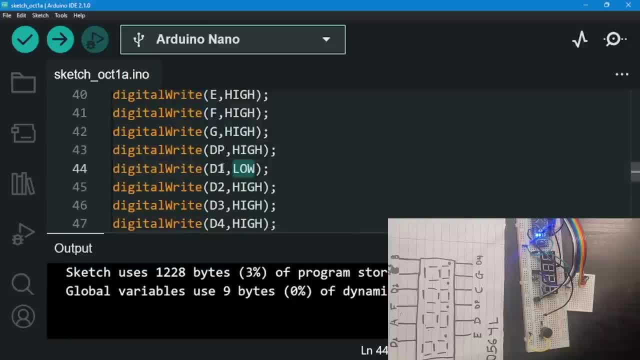 to have what to make a complete circuit. as soon as we turn this all of it to high and then we turn this to low, we basically mean what we cer羅 check si-mi-ni, a multi period, 17 myon-str from ac for stn Sorin. 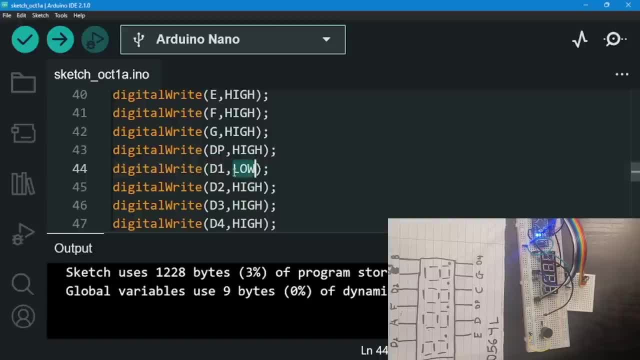 We create a five-volt-to-ground type of circuit, a complete circuit. Okay, now I'm going to set every other to what To high. Let's see if I don't set this to high. Let's see what happens if I don't set this to high. 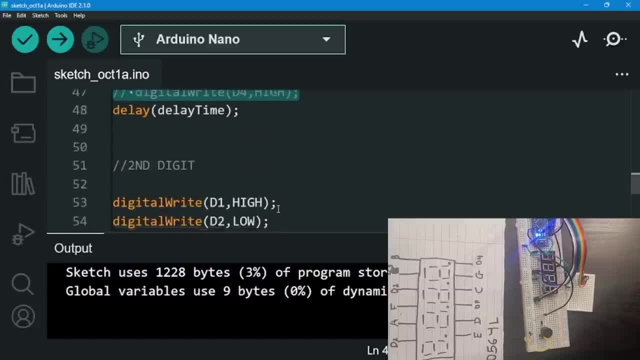 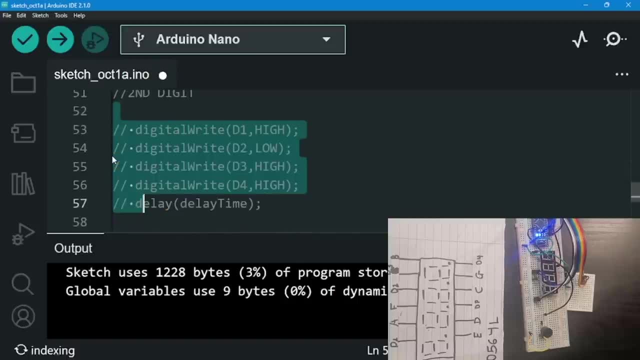 Let me just comment this out. Let's comment actually the second digit too. Let's comment everything and let's just focus on this one. Let me just do that. Let me just comment everything and focus on the first one. 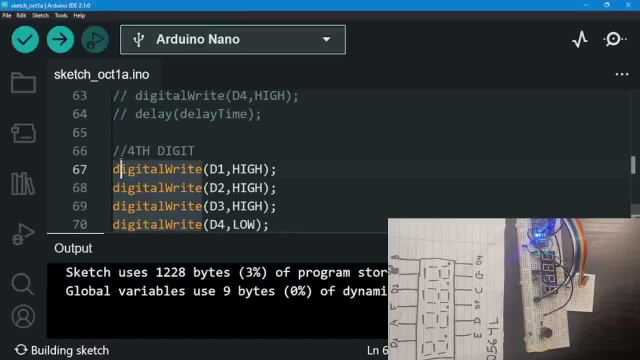 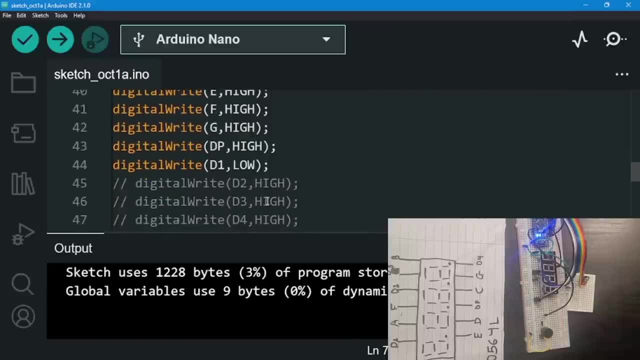 Okay, and I'm going to get back to them. Comment it out. Comment it out Now. only this one should be working. Then I say what? I set this to low. but let's just say I forgot about writing these again. 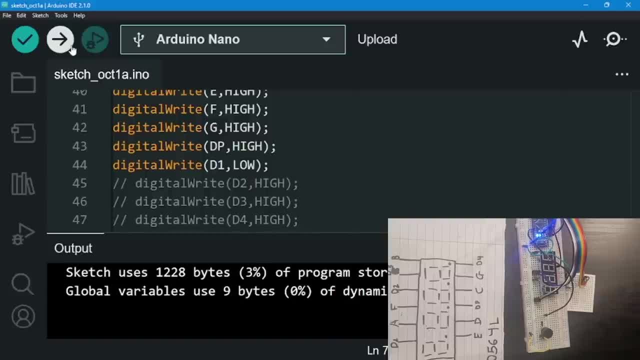 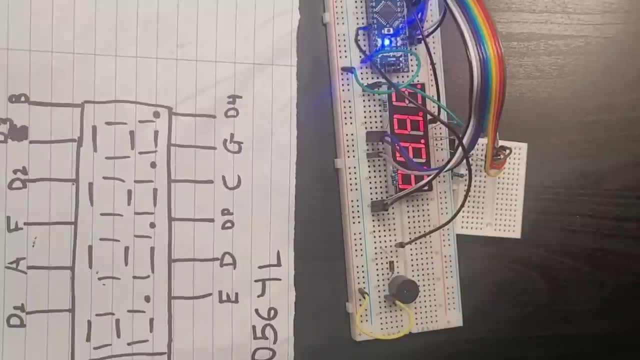 I just only focused on D1 right here and forgot about these. Let's see what happens. Okay, should be done compiling and now it should be uploading. Can you see it? Almost all of them are lighting up, as you can see. 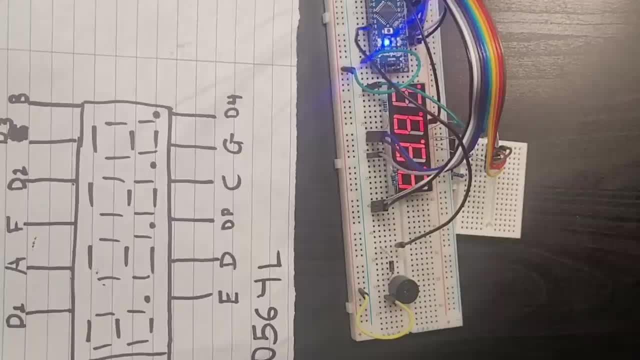 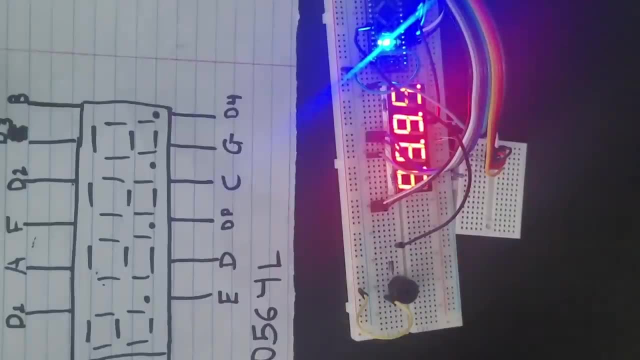 but obviously there's a problem right now. The problem is it's not consistent. I mean, let me just turn off the light so you can see it way better. Some of them- again, what light up Bright, and the other ones are just dim. 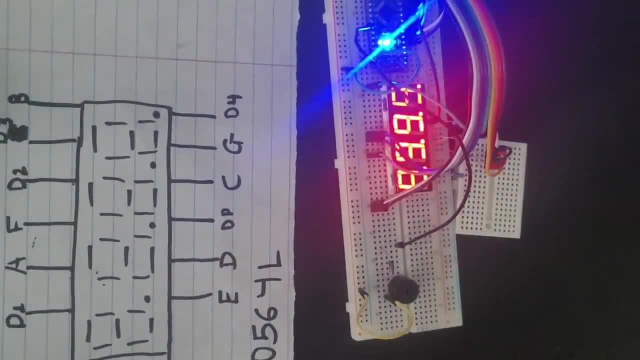 When you look at them, other ones are just dim. I don't think you might notice it in the camera, but when you look at it in real life, it's just the, for example, the four-digit right here is very, very dim. 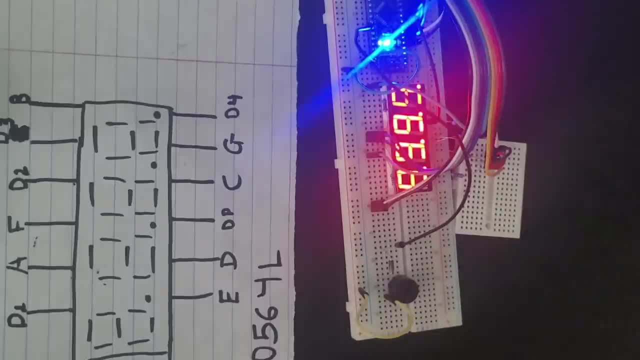 Okay, and obviously they represent what? the same character over and over again Right now. I just wrote down eight. I wanted to write down eight and they represent the same character. I wanted to have this. This is not lighting up. 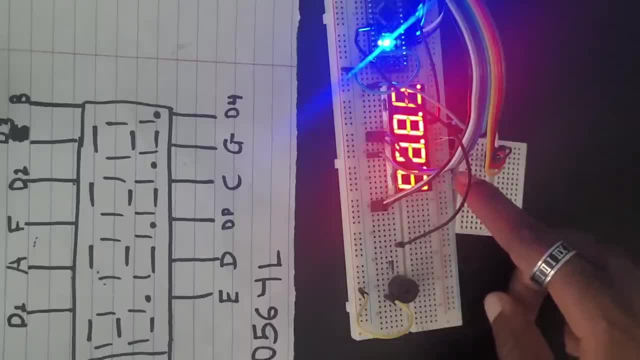 Okay, this is not lighting up. We have to fix this one. There we go. Let me add that segment, The G, which one's not lighting up right now. Right now, the middle is not lighting up. Let's just see what even segment here is. 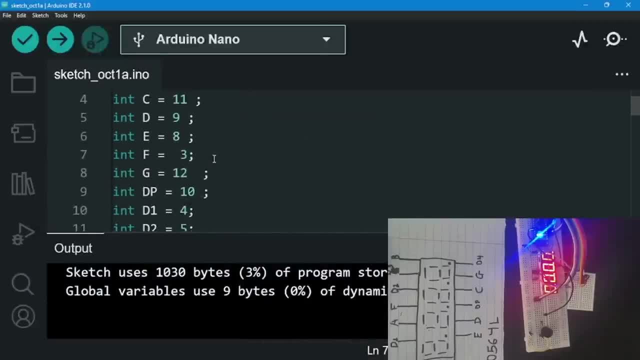 The segment is G. What pin is it? Pin 12.. G is attached to pin 12.. Where is G? G is here, Okay. G is right here, so it should be around here. Okay, there we go. It's a bit of a hustle tool to even connect them. 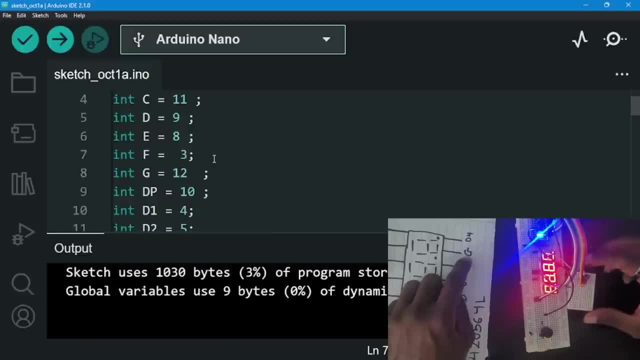 There is a lot of pain even in connecting these. Okay, there we go. Now everything's lighting up, but, as you can see, everything lights up. So, obviously, what should we do right here? We should set everything. what Everything by default is what. 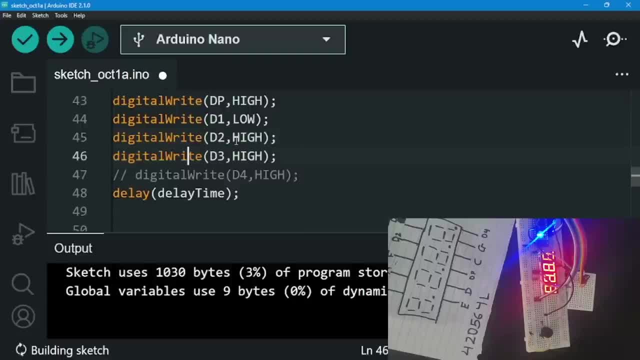 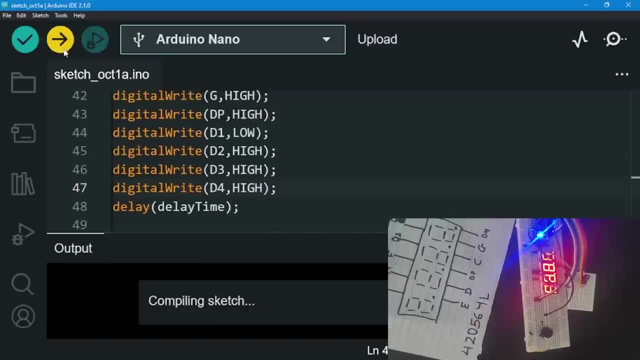 Everything by default is set to low. as we know it, Every pin by default is set to low. We want to set them to high so that they don't what They basically don't, what They basically don't display right here. Let me just set that to high. 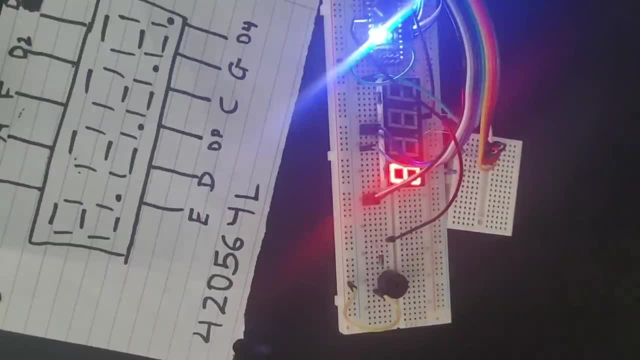 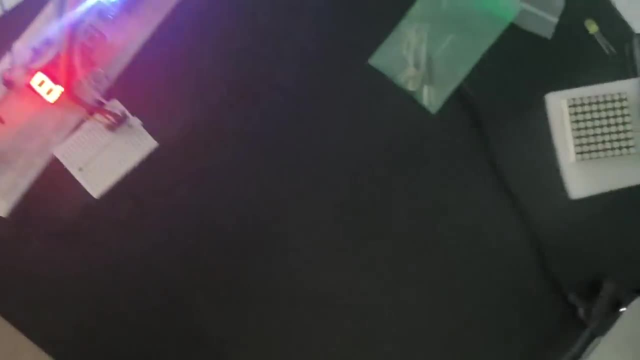 Now only the first digit should be working. There we go. The first digit is displaying really really bright, Nice, Really nice right here. So actually, for you guys to even see it, let me just change the angle again. I'll just keep on changing the angle so you can see it. 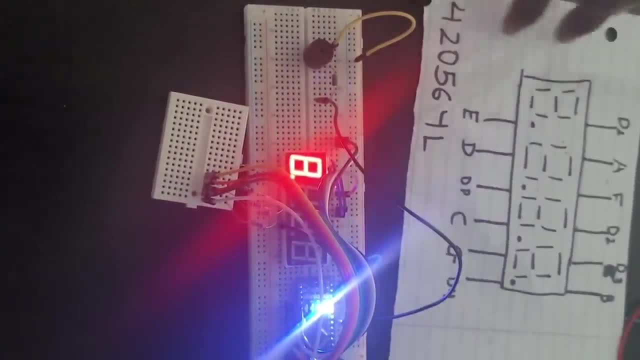 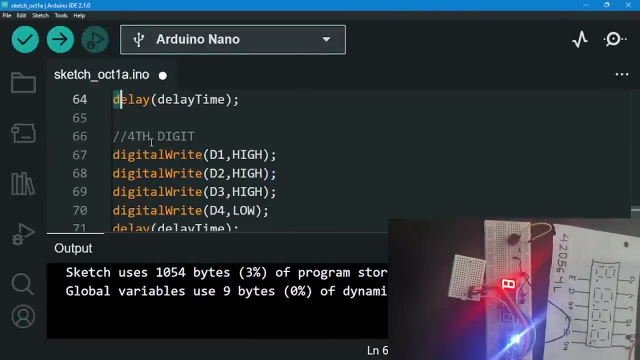 There we go. I think this is better. Yeah, that is better. You can't even see this one too. You can see the. there we go. That's better. Now, obviously, let me just put back the code that I just commented out. 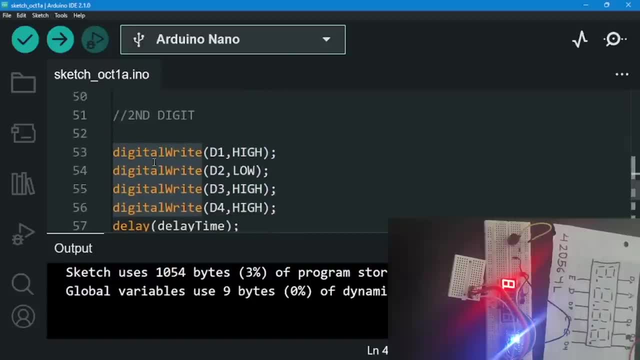 Okay, let me just put that back. There we go, And now let's just upload it. So basically, what happens is what? We set this to low again, then we set this to all of it to high. So basically what? 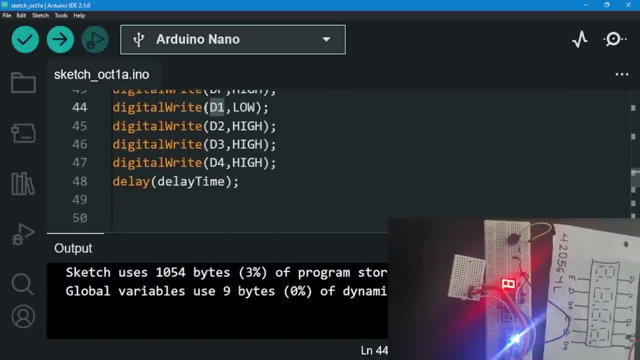 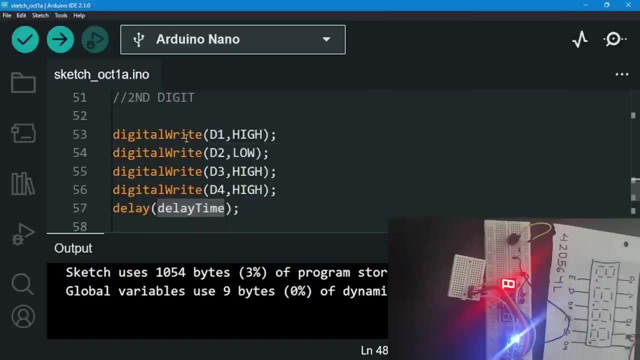 Digital pin one only displays, and then we're going to set it for what? The delay time is set to 100 milliseconds. After 100 milliseconds, what's going to happen is what We're going to set this again, all of it to high the other digital pins. 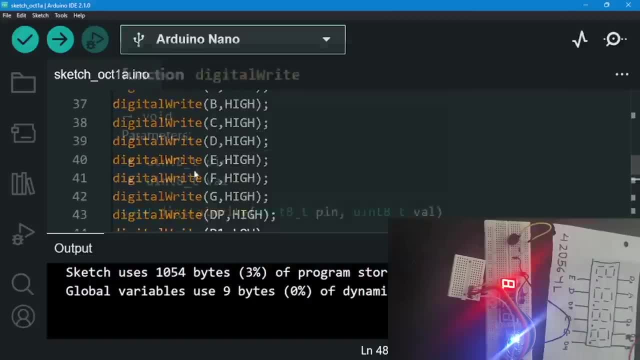 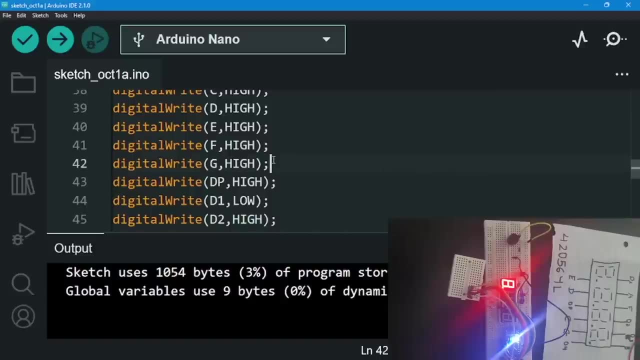 I'm not going to write the same thing over again, because I already set it to high and I want to keep it that way. okay, Because I want to check what everything is working perfectly fine. That's why I'm not going to write this again, because I'm going to be setting all of these. 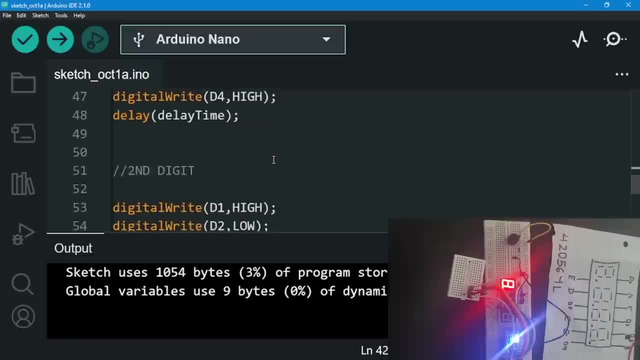 to high. So they're already set to high, so I'm not going to touch them. That's what I want, okay? Obviously, if I want to write down something and stuff, I'm going to turn it off, But now I'm just using it for testing purposes, okay. 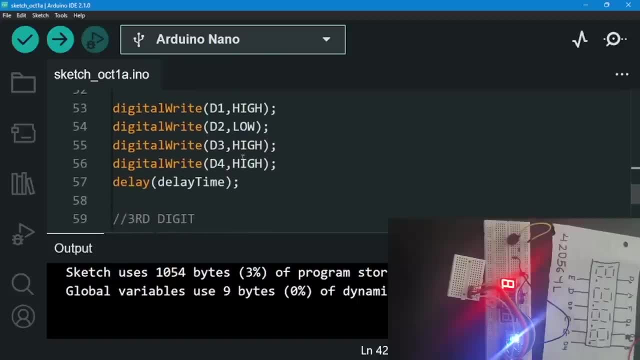 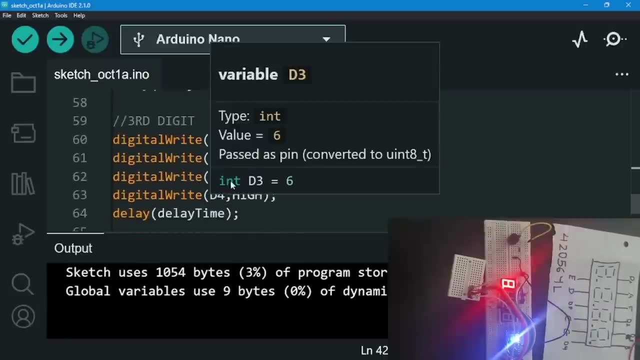 So set this to low for the second digit and set it to what To high and give it a delay time, And then do the same thing, except for digital. what Digital? sorry, Digital. digit three, Again digit three. we're going to do that for low. 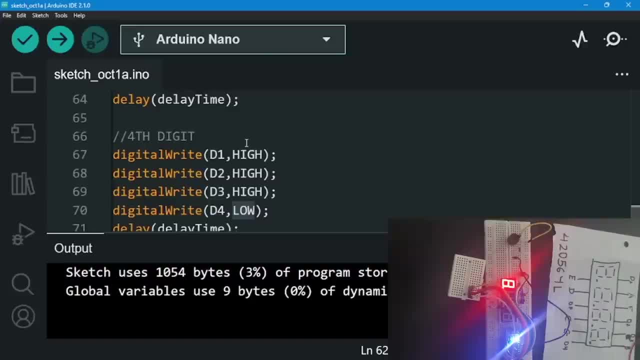 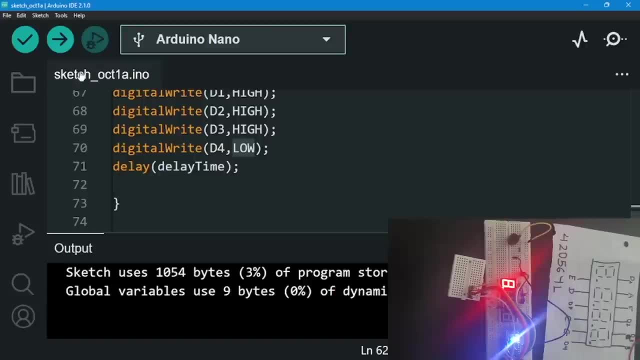 We're going to set it to low and then obviously give it a delay time and then all of it to high, And then finally we got to put what Digit four to low, basically turning on digit four, okay, and then having a delay time, right? 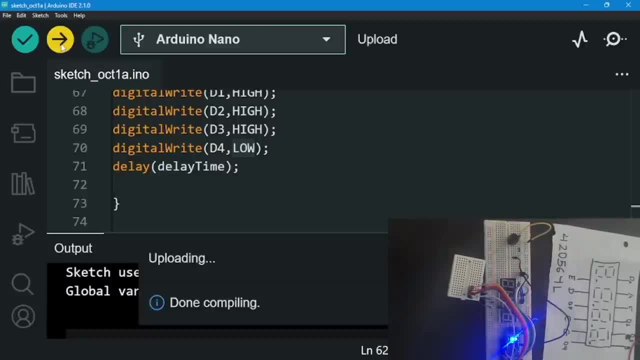 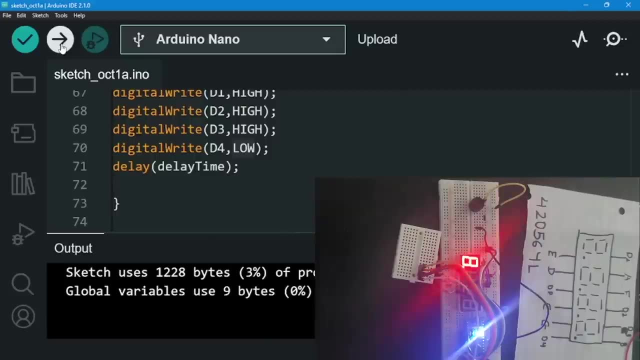 here. Let me just upload this. Let's see what happens. All right, can you see it? It's scanning. Can you see it? It's going eight, eight, eight, eight, eight, eight, eight. I gave it a delay of 100 milliseconds, okay. 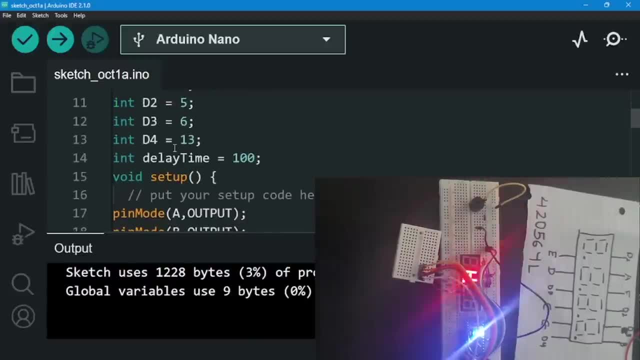 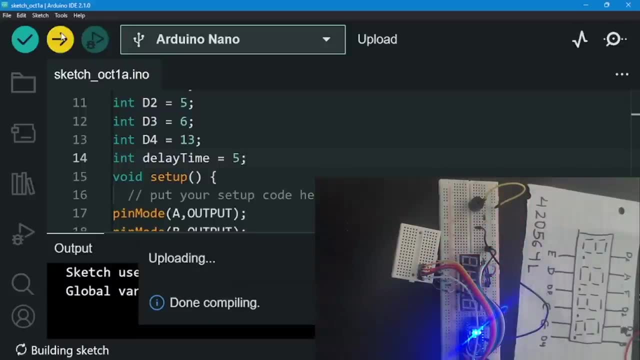 That's how it's working. Let me just set this to again to a very small number, Let's say five milliseconds right now, and let me just upload it. When I do that, let's see what happens When I do five. look at it. 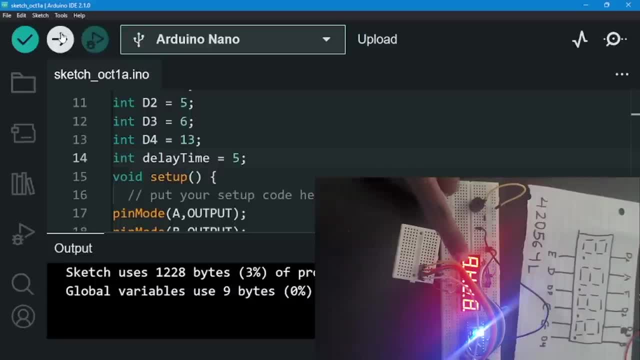 It goes so fast, it scans so fast, it just switches from one digit to another digit so fast that we cannot see it. So we can just see is what We can see is that all LEDs are what turned on for us, for our eyes. 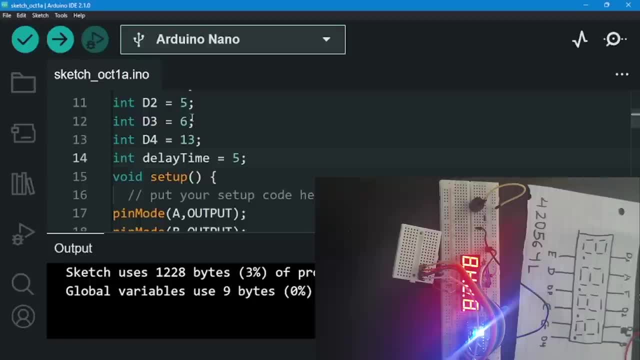 What we can see is what All LEDs are, what Turned on. Obviously, that's not the case. What it's doing is scanning it really really, really fast, Just like how we did when we put it to 100 milliseconds. you can just see the effect. 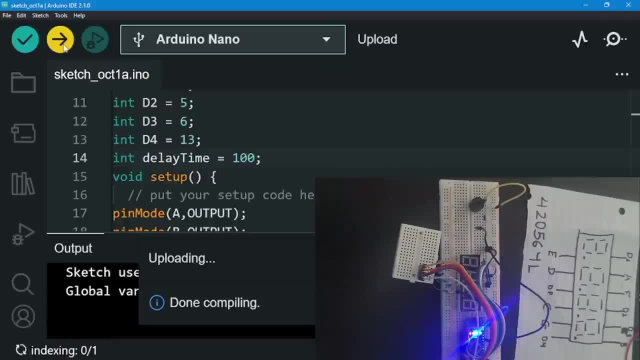 You can see the effect when you put it to 100 milliseconds, scanning it really, really, really fast. Look at it, Look at how it does it really fast, really fast, really fast. Let me just put it to 20 so you can see it. 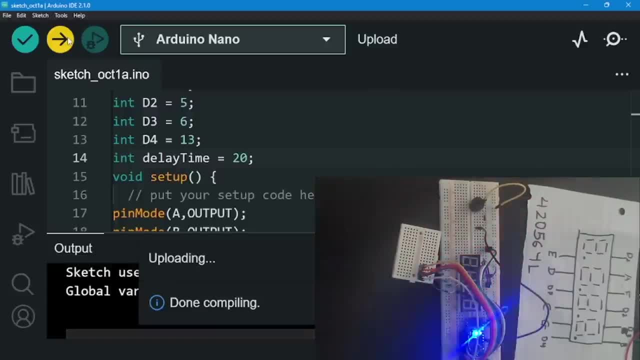 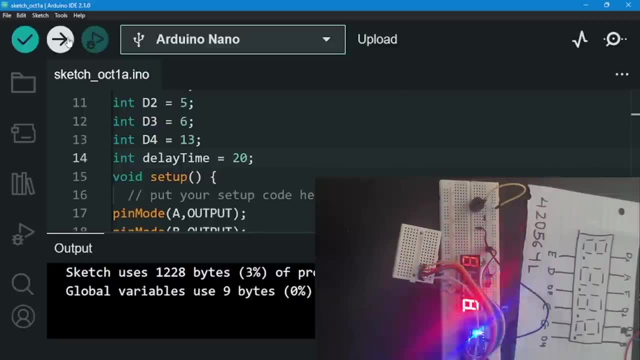 Even Let's go, Let's see how fast it is. Let's go even five times faster and look at it: It's flickering. Can you see it How fast it's going? It's just flickering. We cannot see it. 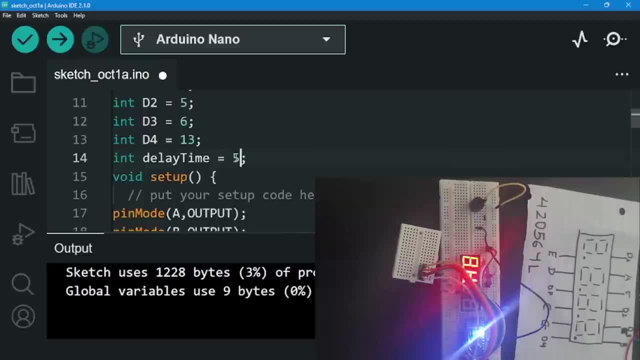 We can see it, It's going so fast. But when you set it to five right now, when we just set it to again five, which is four times faster than 20, when we just do that, look what happens right here. 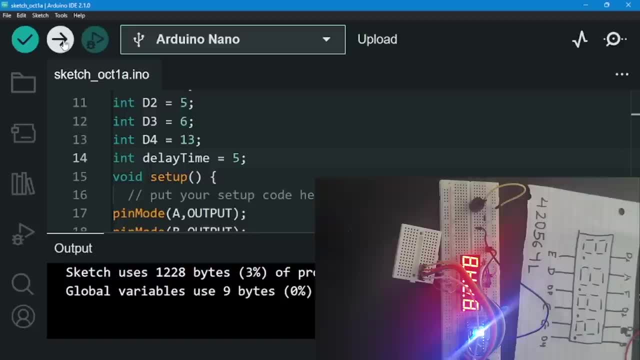 We don't see any interruption, We just see all of them light up. For our eyes, we only see is what All of it is lighting up because, again, our eyes cannot what They cannot comprehend, that type of speed, Okay. 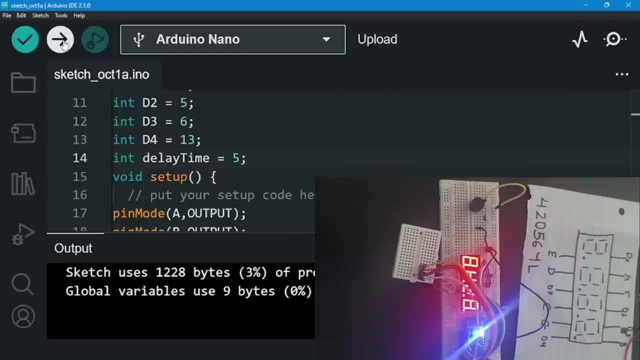 That's all that there is. So everything is hooked up properly and as it should be. Okay. With that in mind, right now, what we're going to do is to make this project interesting is we're going to be using a library. Not only that, too. if you remember when we were working with the, let me just turn. 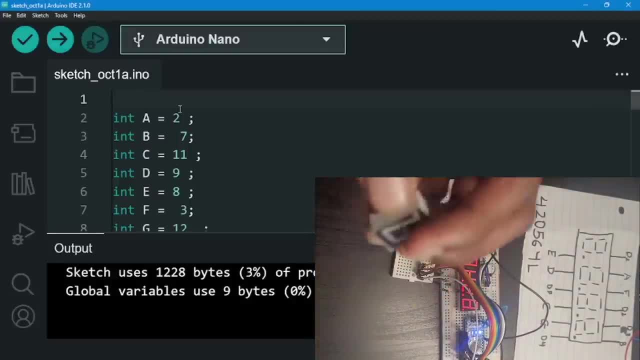 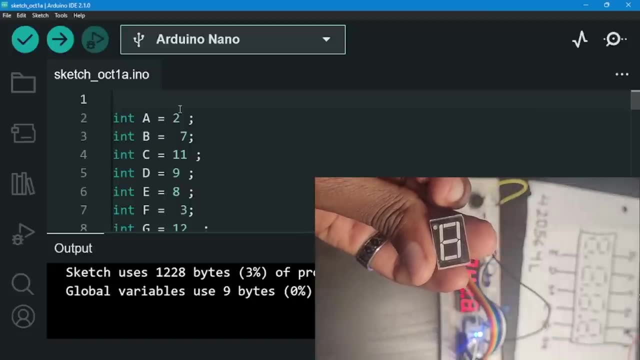 on the light when we were working with the- again, one-digit seven-segment LED display. just focus on the focus on it. when we were working with it, what we basically did was what. If you remember, what we basically did was what. 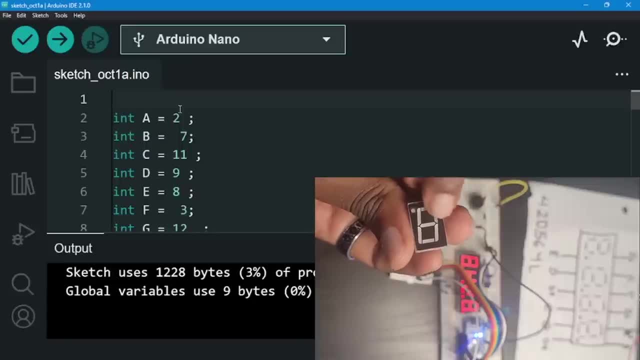 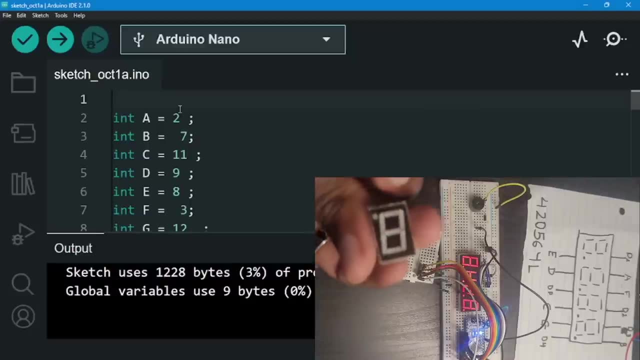 We just used 98.. Seven, six, five, four, three, two, one to just set a timer, to just basically make a timer. We just did was what? Count up to nine? Obviously, this LED segment can count up to what? 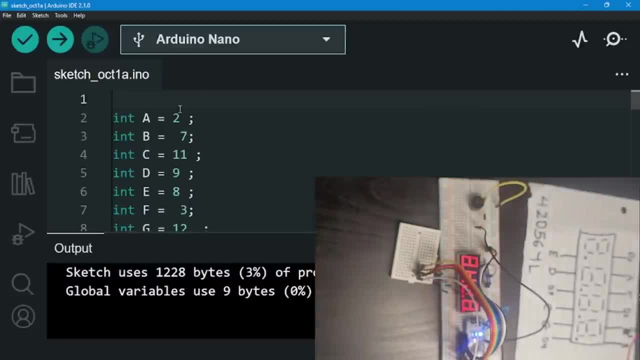 Can only count up to nine, but when we go to the four-digit one, obviously it can count up to what It can count, up to 9,999.. So just think of writing down and setting up all these numbers. Just think of setting up 9,999, going to 9,998.. 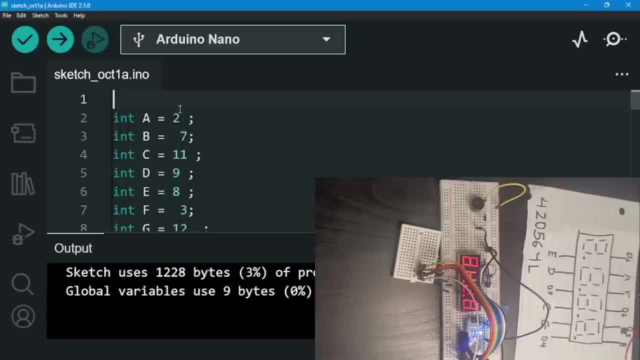 Just think of even setting up all of that. You know It's a lot, obviously. So in this case, it's just way easier to use libraries, so they make our lives way, way, way easier. Okay, So let me just go over to my screen again, and what I'm going to do is let me scroll. 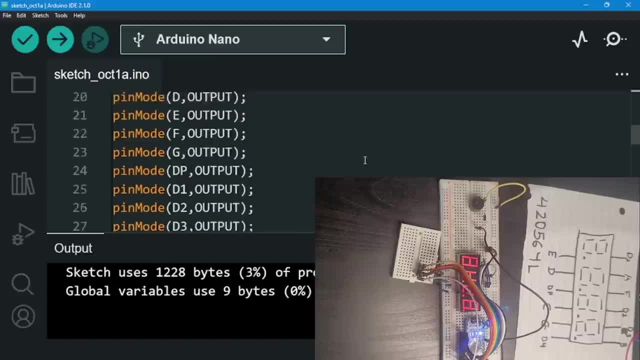 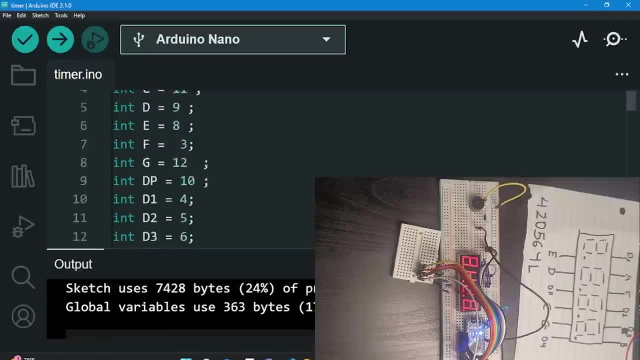 over to my code. I already wrote the code, So again, we don't waste time and we can focus on actually reading the code and understanding the code Okay. So again, I don't want to waste time by typing it, Okay. 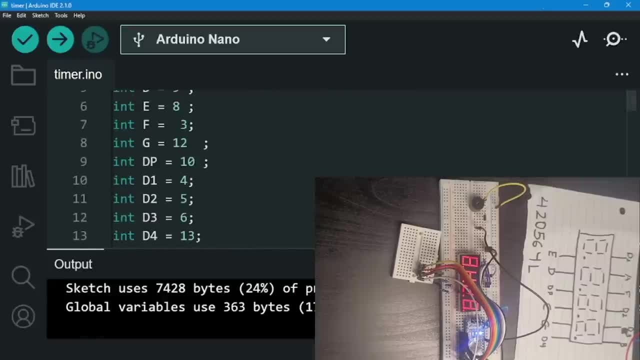 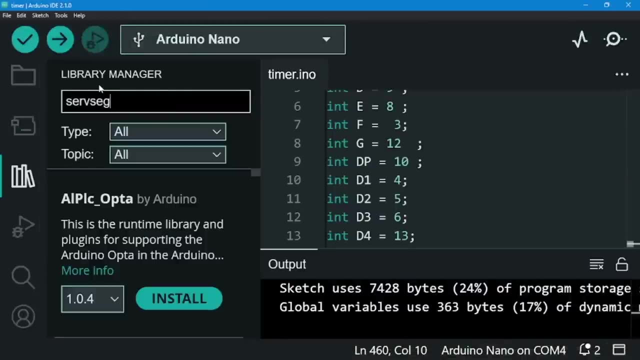 There we go, There's the code. All right, There's the code. So one library that we're going to be using is you're going to go to your library manager and search for SurfSec. Okay, SurfSec, It's literally the SurfSec is literally the library that we're going to be using. 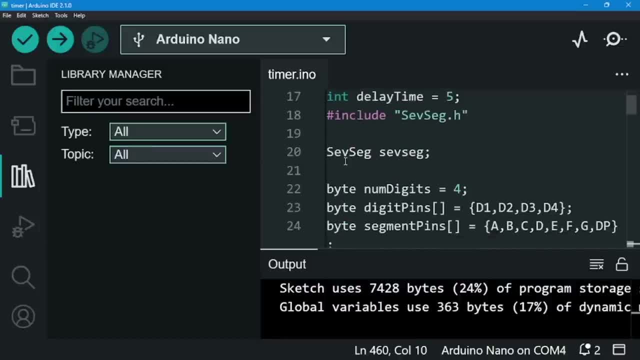 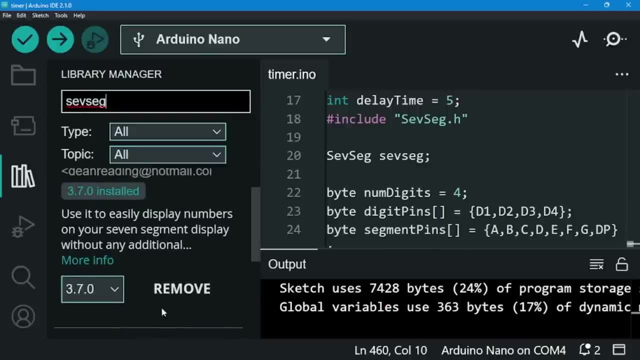 Okay, It's not showing it there. Oh, SafeSec. Sorry, I misspelled it. SafeSec, There we go. Install it right here. You can install it again If you cannot, even if you don't find it on the library manager again, you can go to. 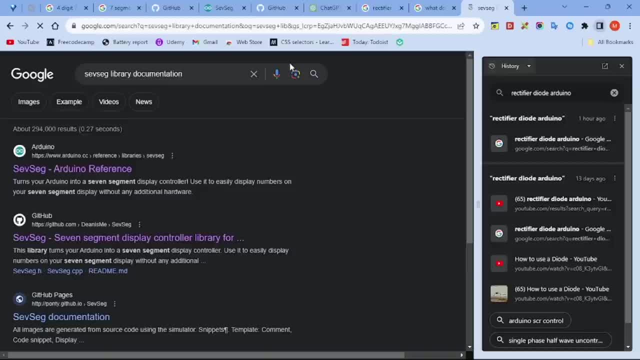 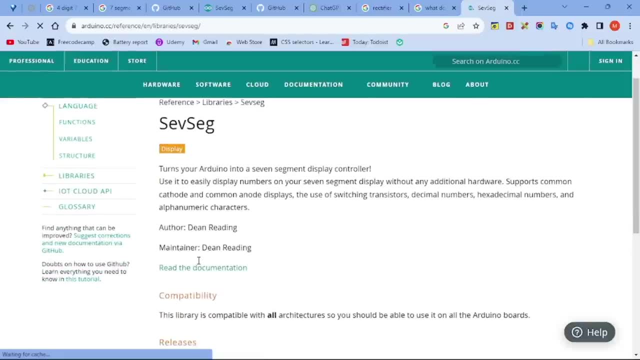 what SurfSec library, And then afterwards, searching for SafeSec, look at it, go to the Arduino page and then you can install it as a zip right here. You can install it as a zip And then you can again add it to what? 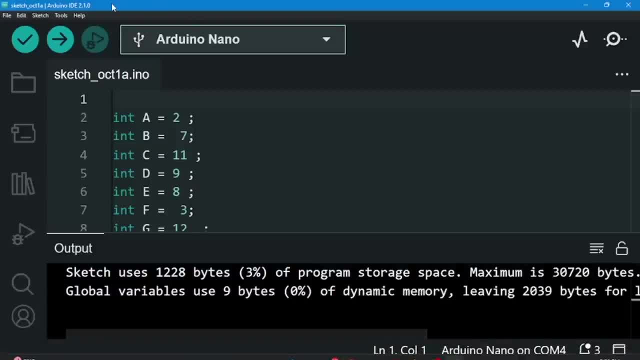 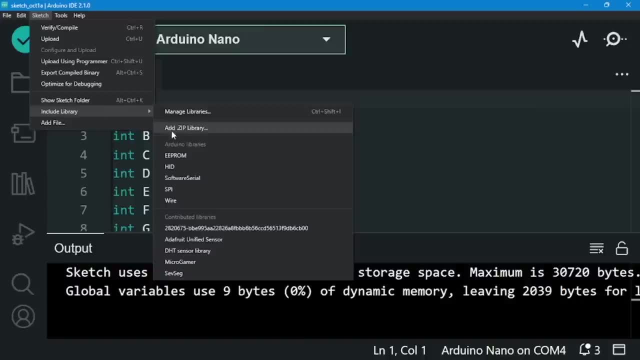 You can add it to your sketch. Basically, I think you guys know how to do it because I've shown you guys. But even if you don't, after you're done doing that, what you do after installing it is you say: include libraries and add, don't zip library. 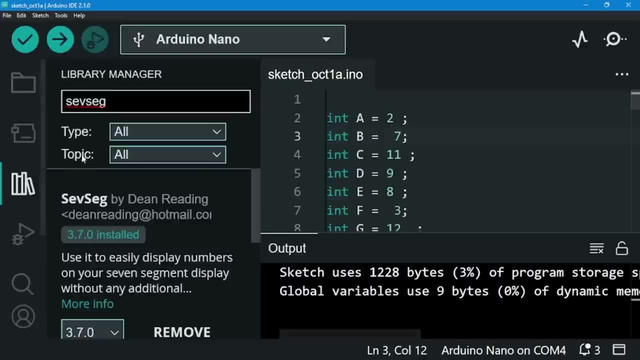 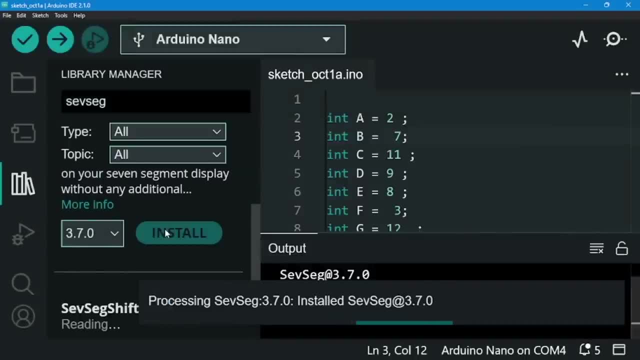 Okay, That's all you need to do, But again, you can just again Download it from here. It's going to be easy Again. let me just remove it for now so that I can install it. As you can see, all you have to do is just tap the install button. 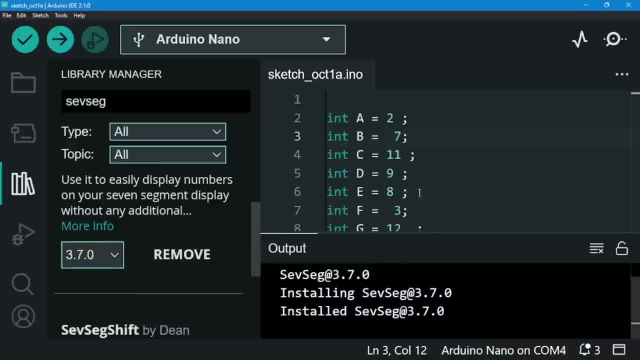 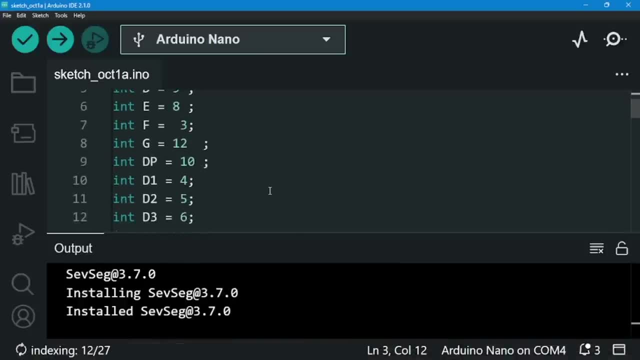 And once you're done, there you go. We're just done, That's all we need to do. There we go. Okay, So the SafeSec library just helps us again work with LED matrices. All right, So what's going to help us is what? 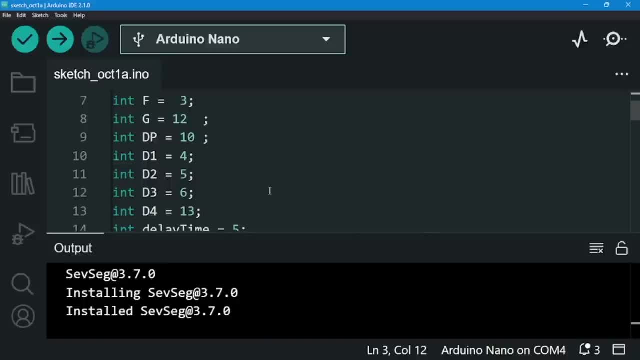 It's going to be working with LED segments right here, So it's going to make our lives way, way, way easier. Oh, I think it's displaying 999.. I'm just going to fix that up. There we go, Okay. 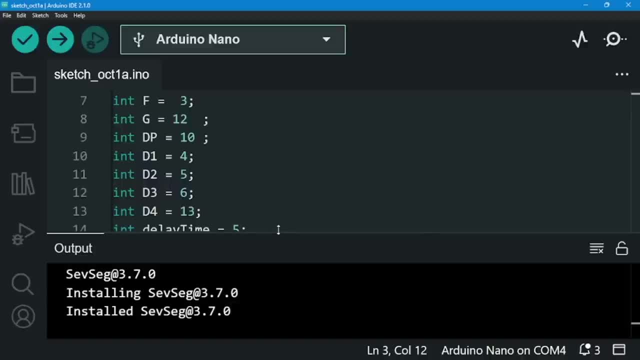 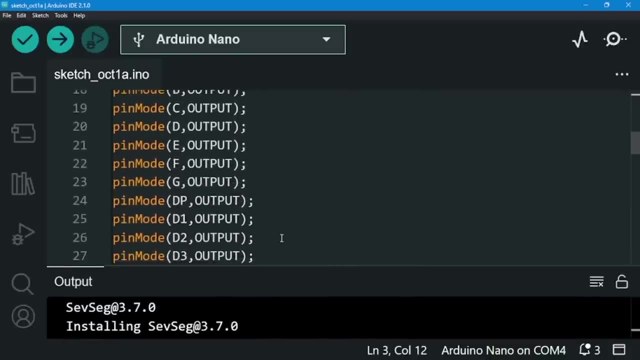 It's going to make our lives way easier. As I said again, using libraries. we're just going to what we're going to focus on: actually work on our project and actually understanding lots and lots of concepts, because they're going to be a lots of concepts here. 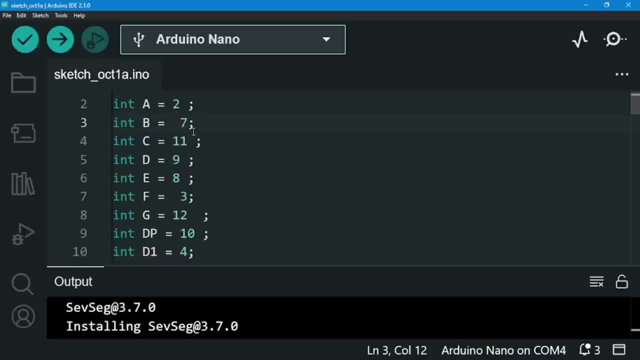 Okay. So what I did again is here and my code. actually, I can turn off the light. No, let me just keep it on Just reflecting. Yeah, Let me just put it down. There we go, Okay. So when it comes to the code, all I did is again. 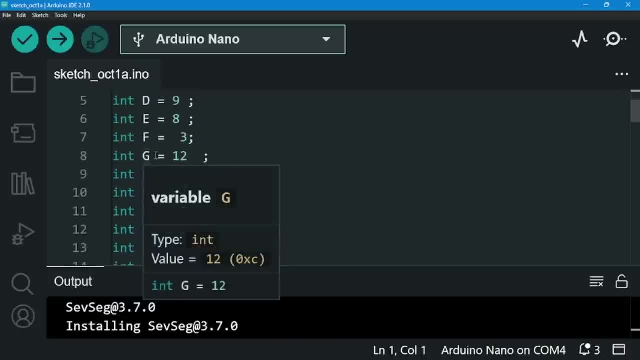 Set up the every segment right here with its respective pin, And then again put again the digital, again the sorry, the digits right here, set it up and I set up a delay time of five, five milliseconds. That's all I did, right here. 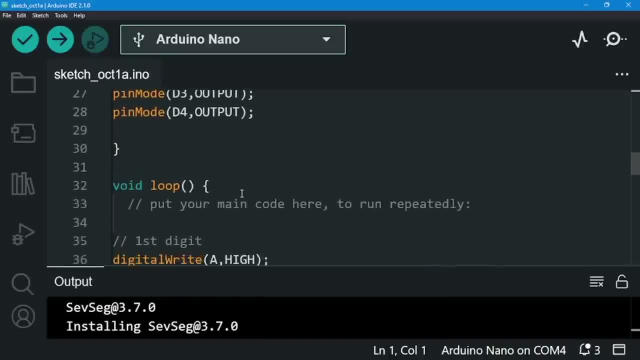 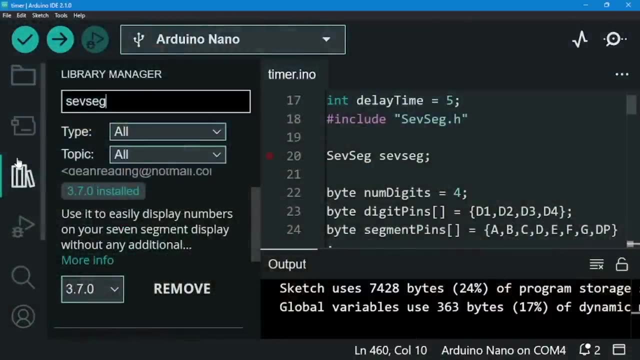 What do we set up? Okay, Wait, this is not supposed to be the. this is not the. well, this is the one that I turned on the old of the second experience. Where's the other one? There we go On the other one. 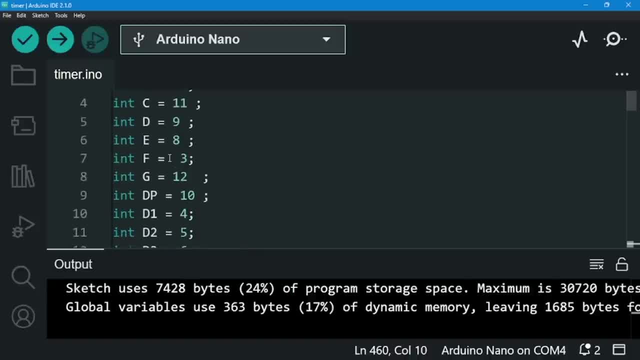 I want this one. There we go, There we go. Well, I did this again. Set up what, Set up every digit, again and again. give it its variable, give it a variable name, And then what I did here is user input. 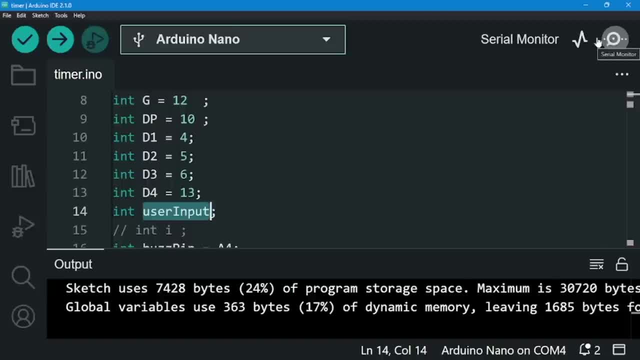 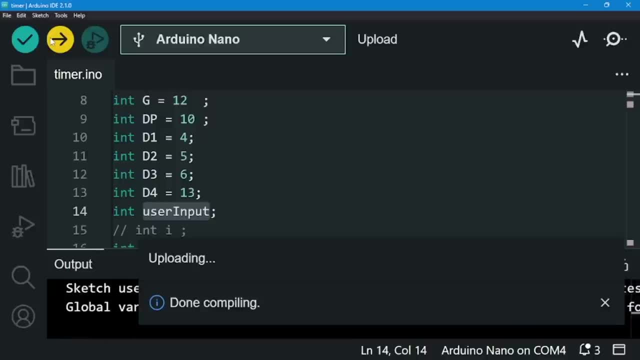 Basically what this program does. let me show you. let me just show you the program running. Let me just upload it first so I can see how the program works. Okay, So it compiles my sketch. Okay, It's done compiling. 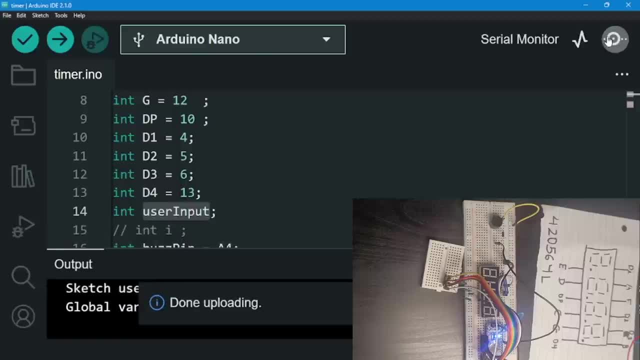 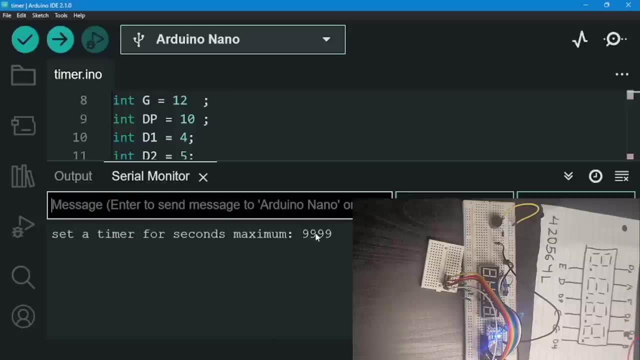 Now it should be done uploading. Okay. So let me show you what happens again Once you're done building the course, what is supposed to happen. So again, we can set a timer for seconds. Maximum is what? 9,999.. 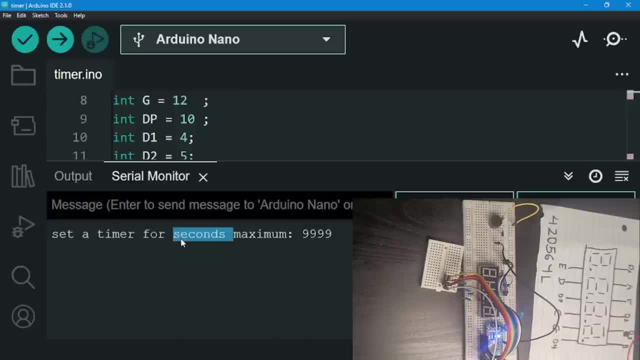 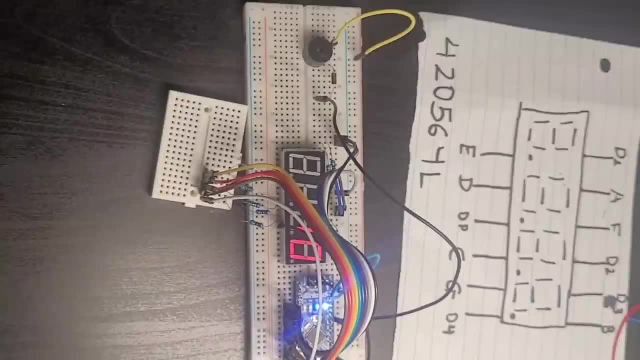 9,999.. So, again, we're going to set a timer in what? In seconds? Okay, So I'm going to set a timer for, let's say, 10 seconds. I'm going to enter it. Okay, After I'm done entering it, it starts counting to 10, goes eight, seven, six and you can. 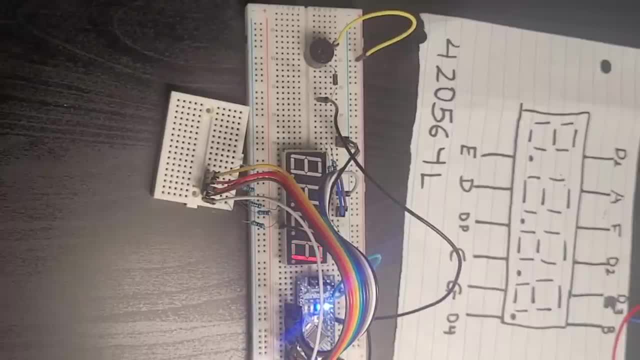 see five. It's going four, three, two, one And the buzzer should be ringing. The buzzer isn't that loud. Let me try it again One second. Let me try it again One second, One second. 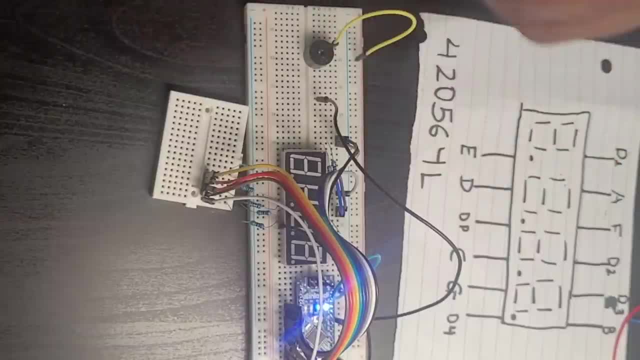 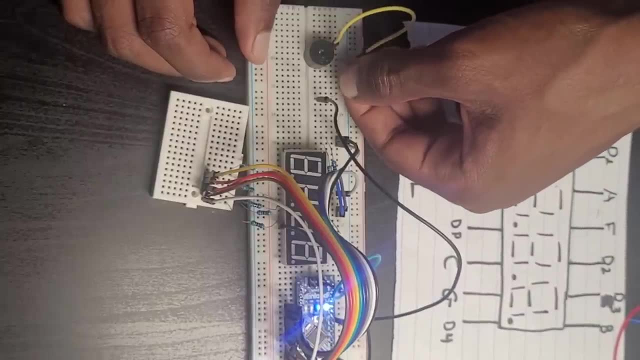 One second again. Did I flip it? Maybe I should flip it. I should flip my diode, because you cannot hear anything. Maybe I again put the wrong direction on the diode, because it can happen. as I said, Let me just get the positive. 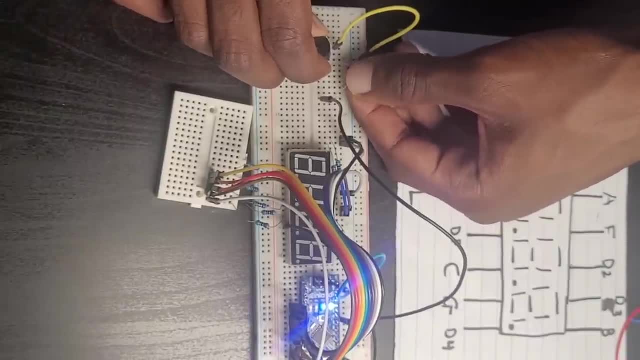 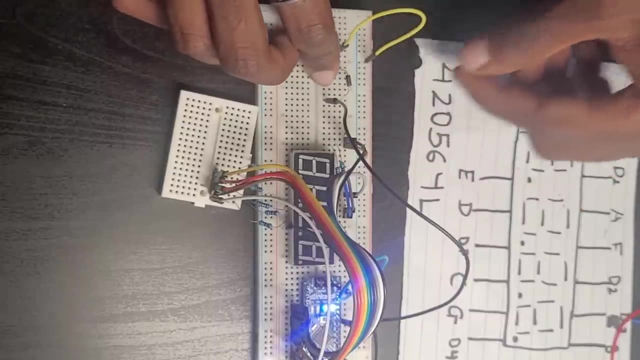 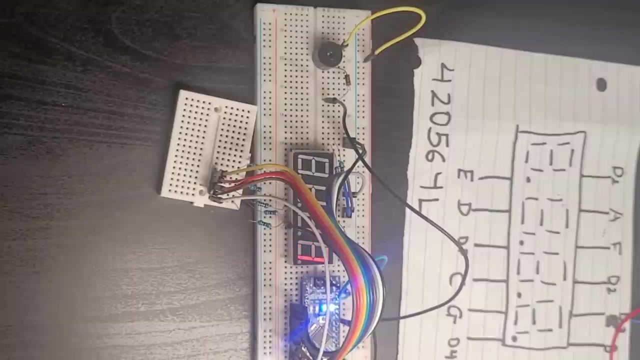 Get the positive of this Right, The positive. There we go. I think it's the opposite direction, so we're not hearing anything from the buzzer. Let me just say two seconds now, two milliseconds. We're totally not going to hear anything. 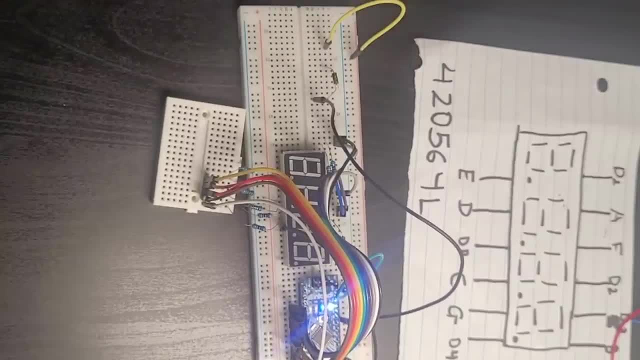 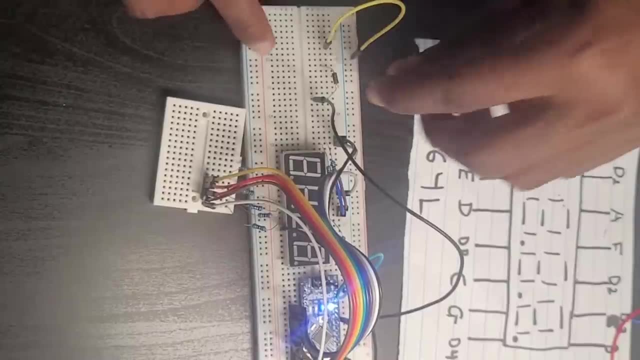 Okay, I'm using an active buzzer. Okay, there we go, And let me just check the polarity of the active buzzer. The positive is supposed to be here. Let me just change the direction. here too, I think it's direction. 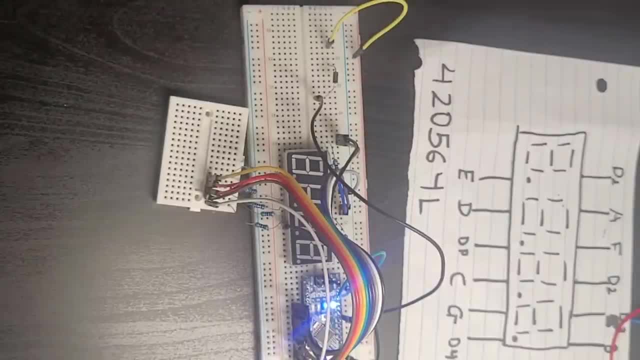 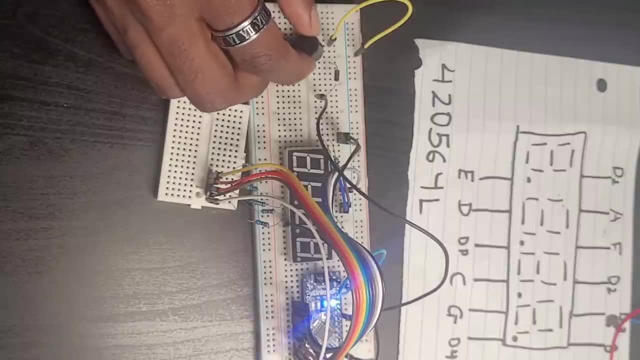 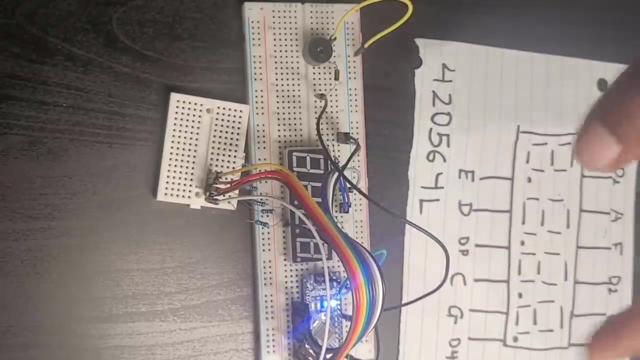 Right, The positive is here. The negative should be right around here. Okay, the positive is connected to the negative. This is connected to the negative terminal, basically the GND. Okay, and then this is going to be connected to analog pin 4.. 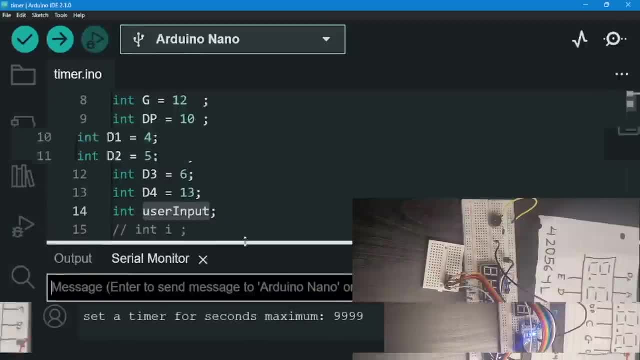 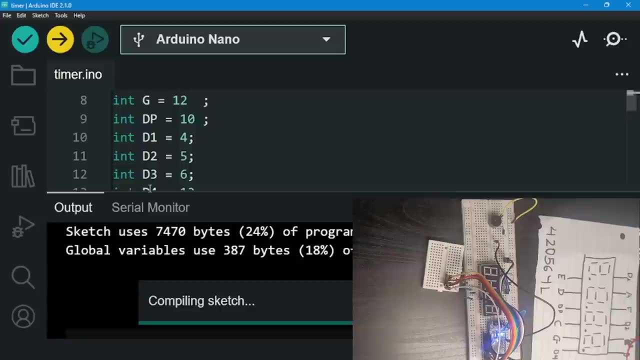 I set it up as analog pin 4.. Let me just check it out. Buzz pin is set to, as you can see, analog pin 4.. Let me try to upload this code again. This should be the uploading. Let me turn off my serial monitor first, though. 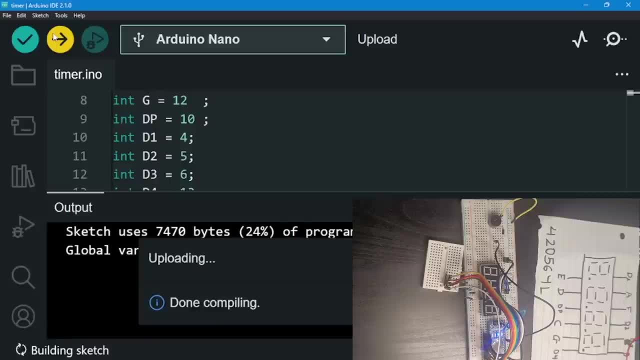 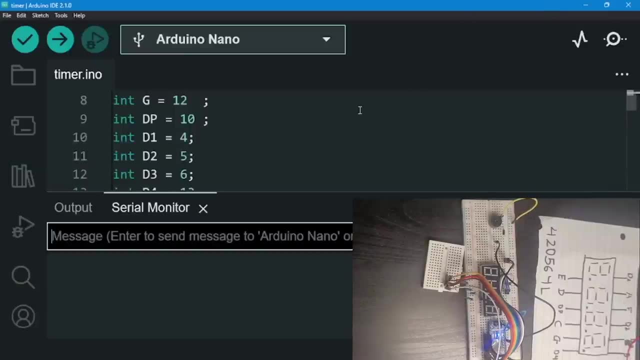 Let me first turn off my serial monitor before uploading it. Okay, it's done compiling. Okay, it should be uploading. All right, there we go. Let me just again set it for three seconds. Counts three, two one. 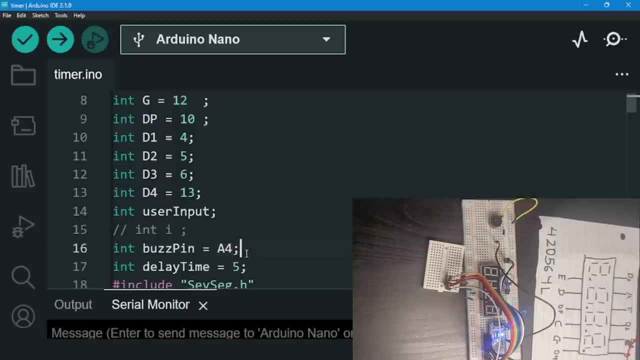 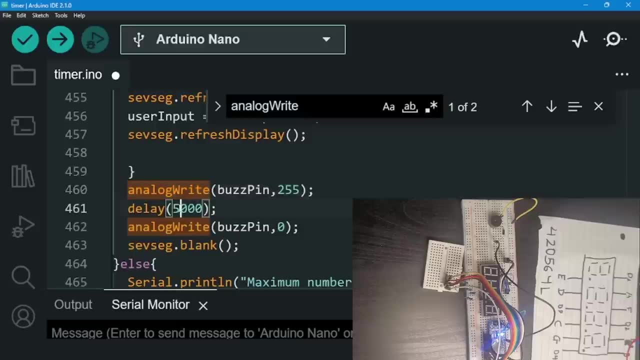 Okay, I think the problem is let me just go over to my try to find analog right. Okay, let me just set this to five milliseconds, This one to 255,. yes, Basically five volt, 255 volts, yeah. 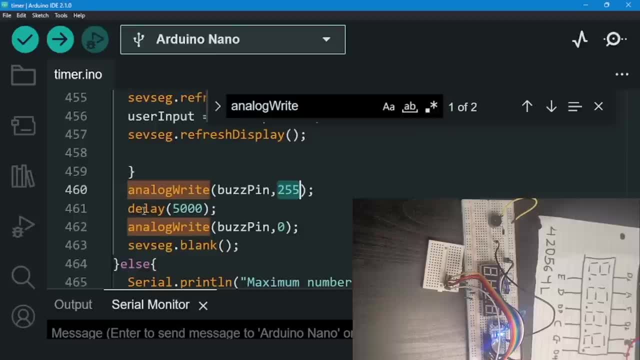 And it turns off after five seconds of what? Five seconds? of playing a timer. Let me just do that Again: turn off my serial monitor fast before it's done uploading. There we go. Let me go back this code. Let me go up. 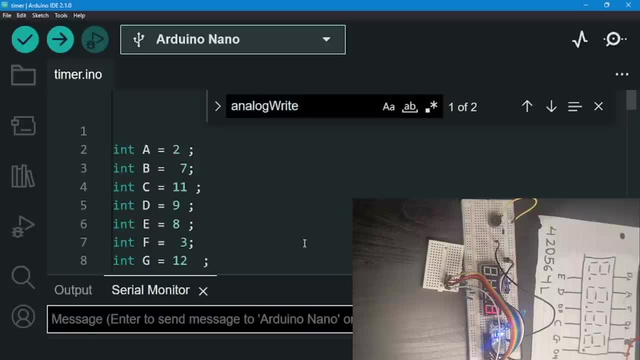 Now let me go to my serial monitor. Let's set it three. It should be working. Come on, Can you hear it? Ooh, I think you can hear something, but it's not the best. Okay, I think it's because this one is not connected properly. 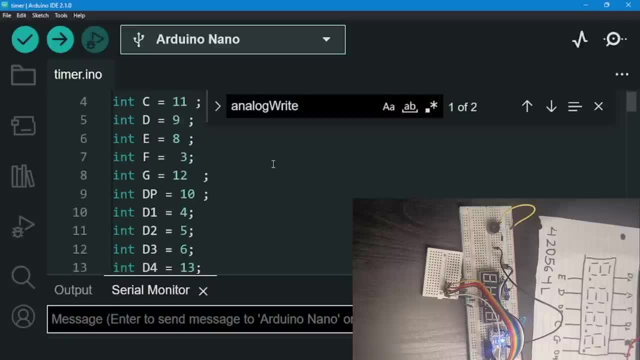 I think one of them is not connected properly. You know what? So what I'm going to do right here is again search for analog right command. Let me just turn off this analog right. Let me just when it turns it off. 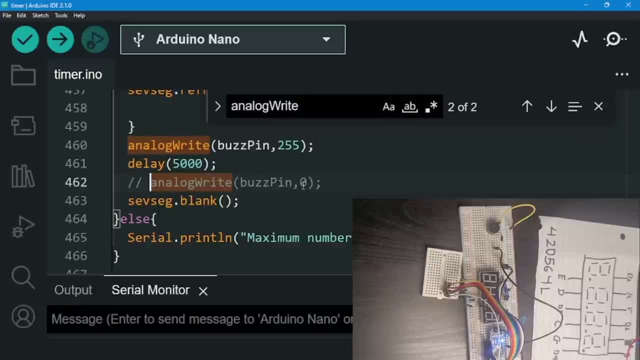 This is basically turning off your what. It's basically going to turn this off After five seconds. it's going to turn off what- Our buzzer. So let me just turn that off. Let me try to wire it up properly. I think it's the wiring that's causing the problem. 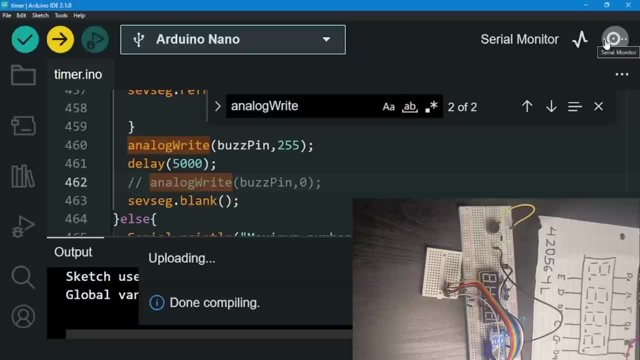 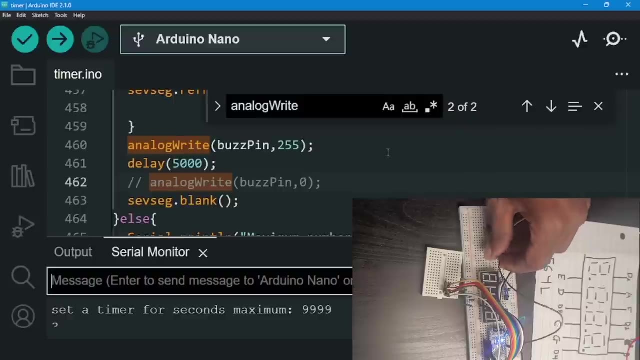 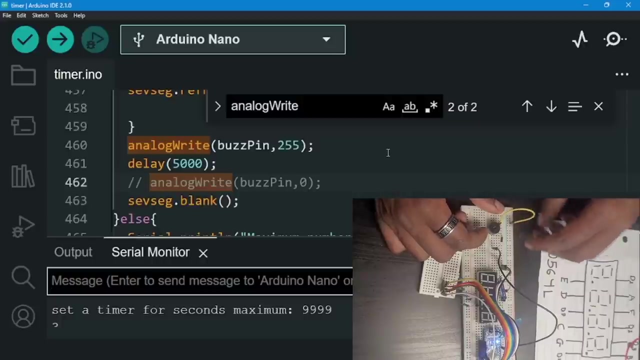 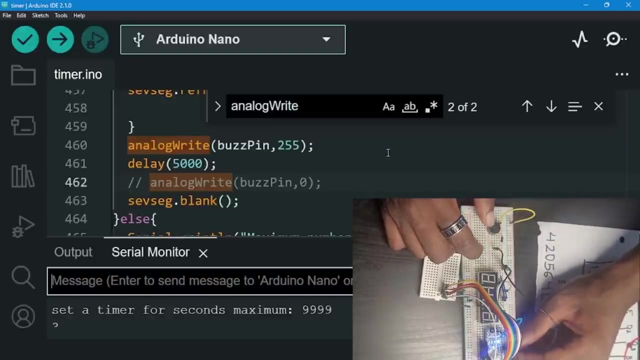 Let me upload this code first, And then let's try to again use the timer. Let's just do that. Done compiling, uploading, and it should be done uploading. Okay, let me set this to three. Okay, now we can hear it continuously. 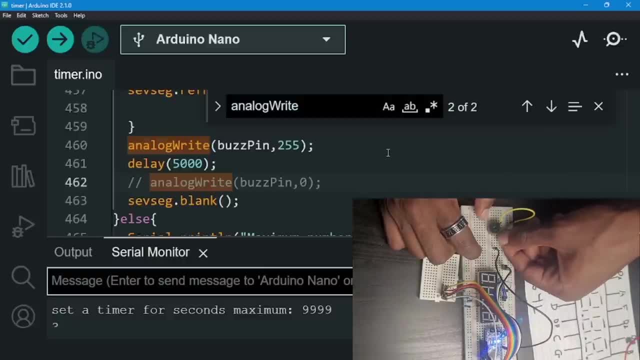 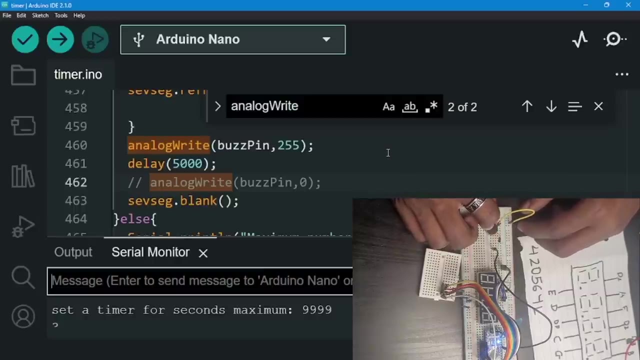 This is correcting the analog pin for it. You can hear something, can't you? Can you hear. So what happened again? What did I say right here? I said that when we're using what, When we're using diodes, what happens is what. 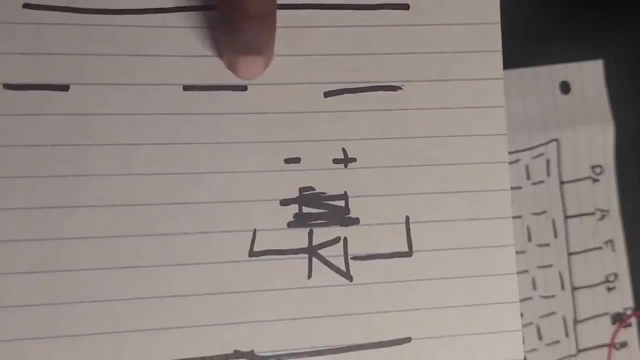 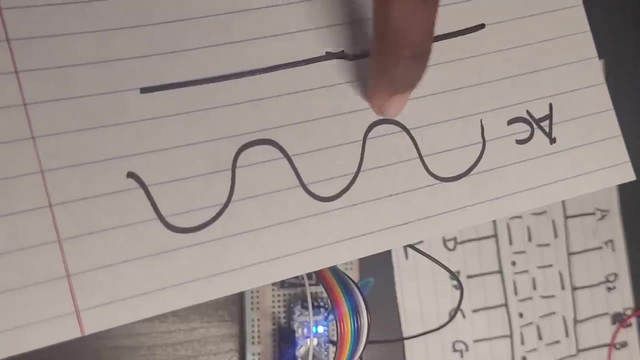 We hear it half the time, Basically, Okay, we hear it half the time because, again, when it comes to each circuit, it goes back and forth, So it's going to only work what In one direction, Let's say the back one, works. 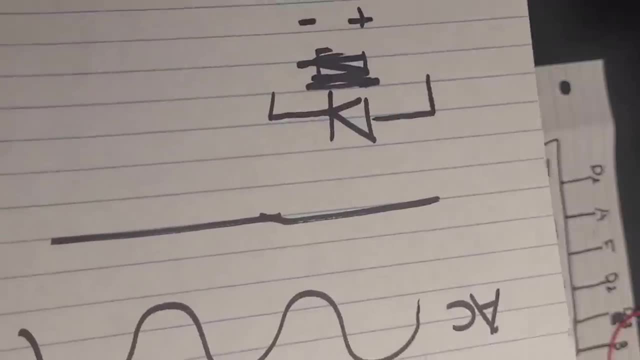 Okay, let's say, the back one works, The fourth one doesn't work, Okay. So basically we're going to hear it. for what? For half the time? Okay, So we're basically hearing it. as what? Can you hear it? 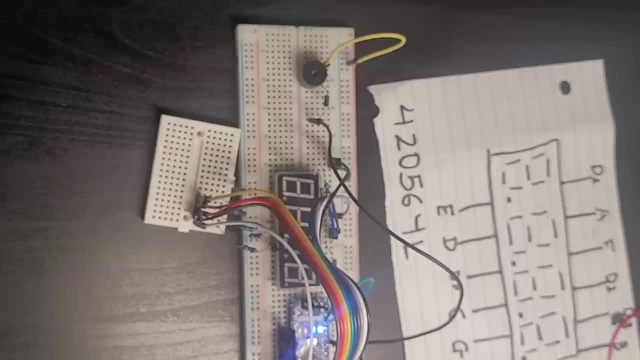 It's not like the normal active buzzer sound, but it's creating a sound. Why is that? Just think of it as if you're using a delay of what? Five milliseconds, and then what, Giving it an off? Okay, Just turning it off. 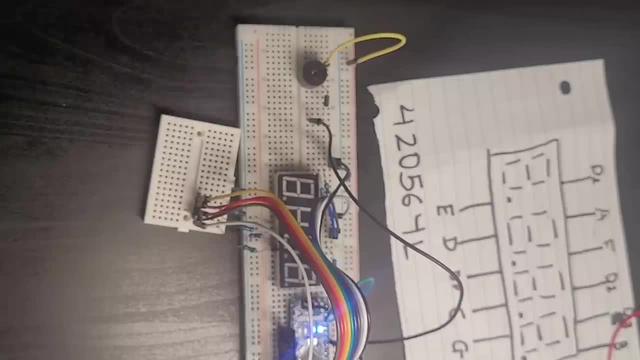 On off, on off, Keeping off doing it for what? For over what? Half of the period of time? Okay, Just think of doing that. It's basically that Okay, Because it's turned off. for what? For half of the time. 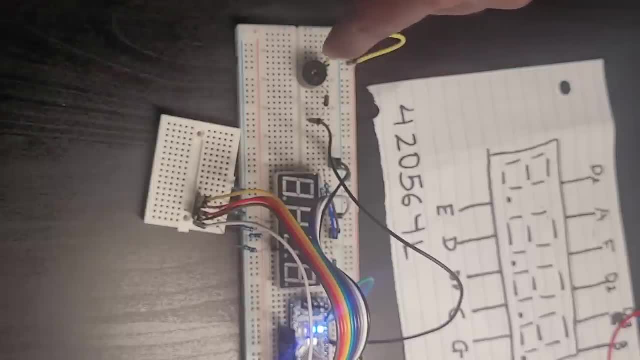 As I said again, when it goes to the other direction, when the current reverses in the other direction, it's not going to go to what? To the buzzer. Why is that so? Because we have a what? We have a diode. 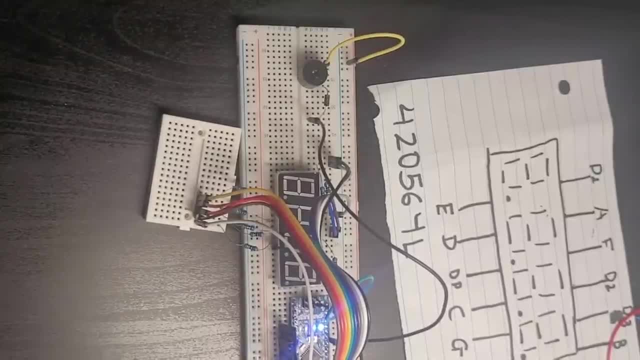 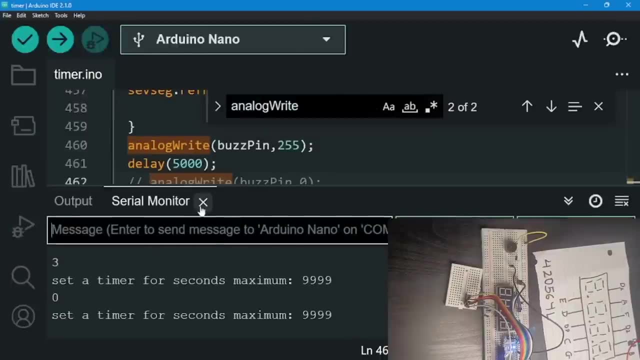 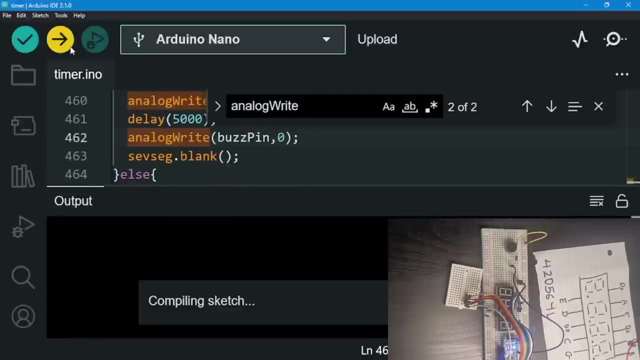 Okay, Let me just focus here. There we go, It is working. Okay, Now let's focus on something else. Let me just turn off the serial. Let me just actually upload it again. Let me first turn this on, so that it turns it off after five seconds. basically like: 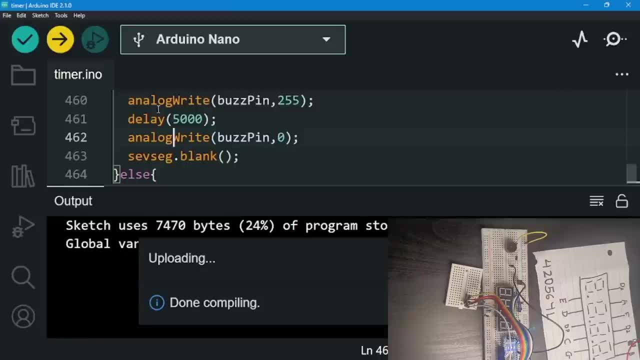 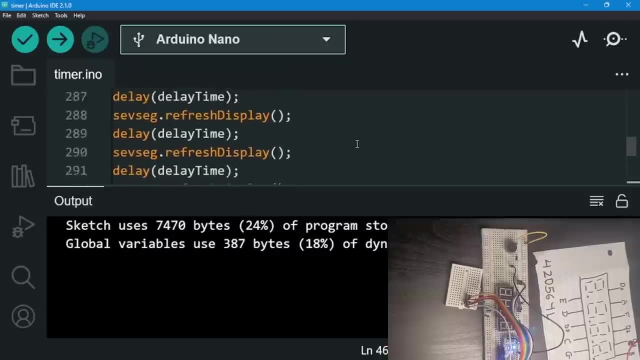 how a timer just turns off after a while. It's going to turn off after five seconds. Okay, That's the code, right here. Let me just go all the way up and let's start actually analyzing the code, because it does work, Okay. 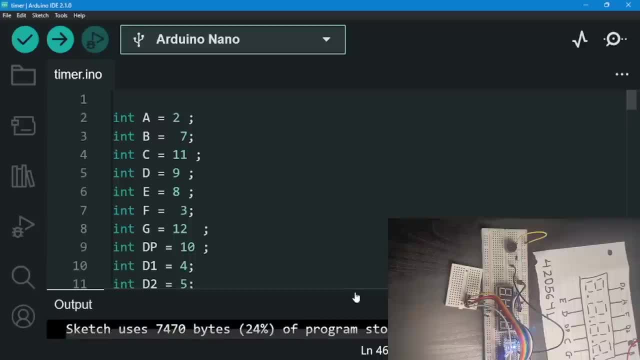 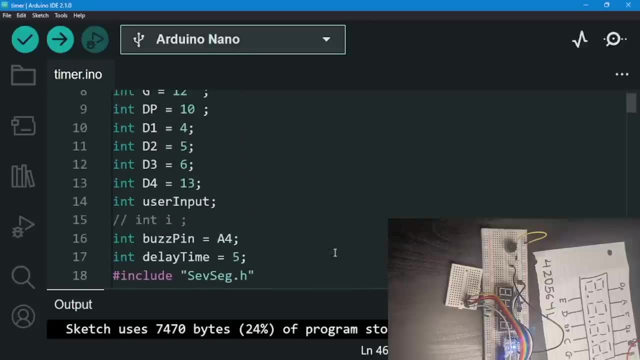 I know it might seem a lot of code, but I'm just going to explain to you what I just did. This is a copy-paste, so don't get intimidated by the amount of code that there is here. Okay, So user input is what? 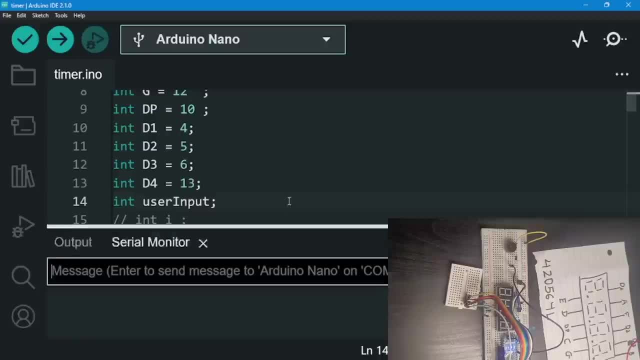 User input is basically the amount that we're going to be receiving from what? From a user right here. I'm going to save it. So, for example, the number we're going to be receiving here- If it's a 30, it's going to be what. 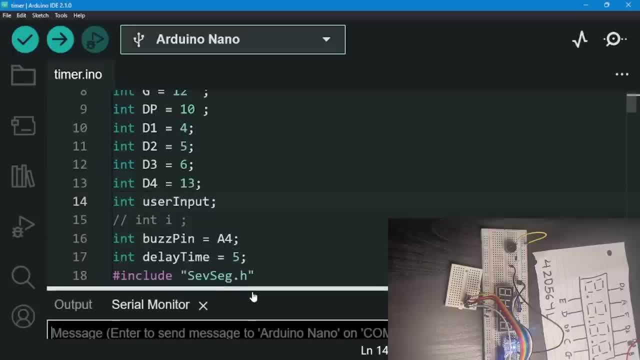 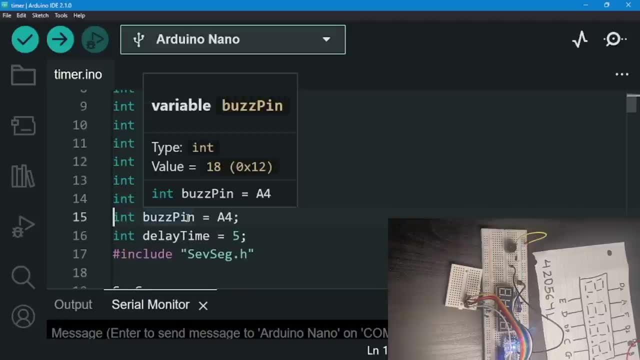 User input is going to be what Set to what? The 30 right here, Okay, It's basically that. Okay, This code is useless right here, so I just removed it. And there is bus pin right here which is going to be set to A4. 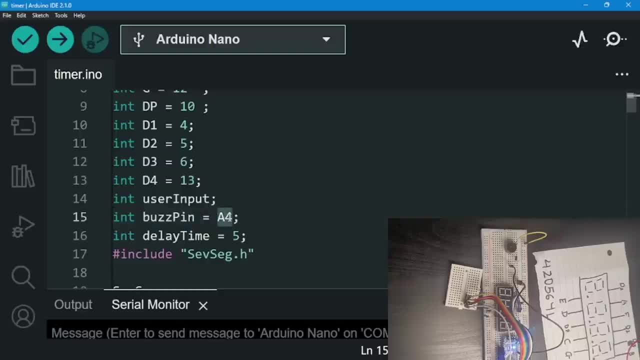 Again, I'm going to be using this obviously for my code, I'm going to be using this obviously for my buzzer. It makes sense. And then I'm going to set there a delay time of 5 milliseconds. 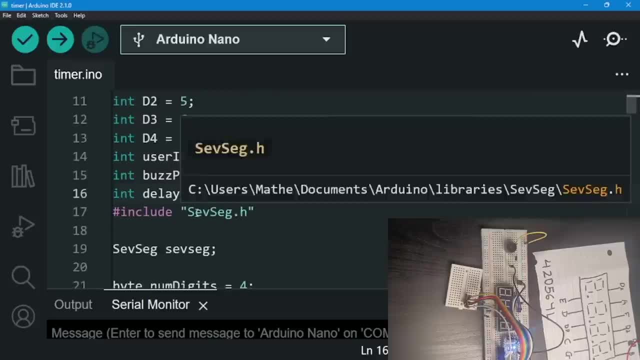 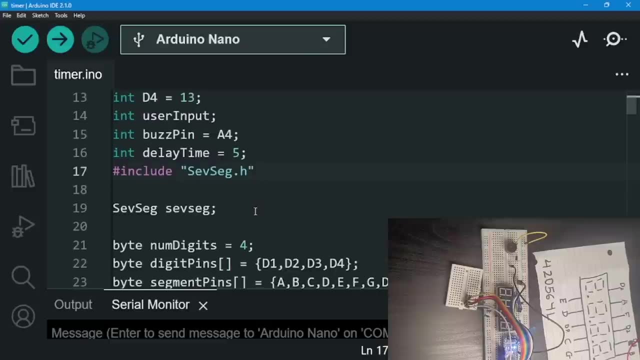 Okay, Then I'm going to what I'm going to include the Cephseg library right now, the one that I again what Installed in the library manager. I'm just going to include it right here, And right here it says what. 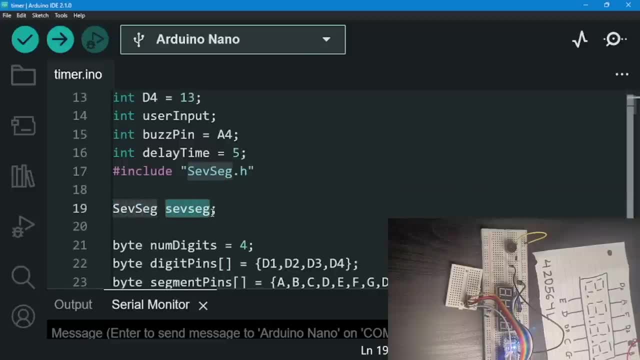 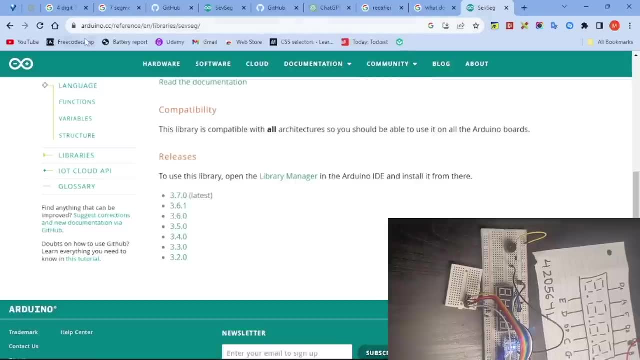 Cephseg, Cephseg. right here Again the capitalization matters. Okay, Again, you can read the documentation for yourself. You can just say, you can Google it yourself. Say: Cephseg documentation. right here, I already Googled it. 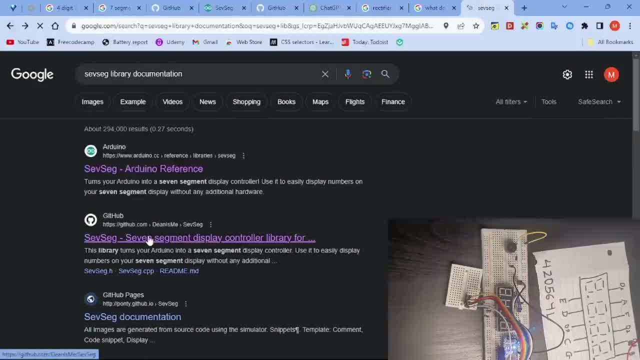 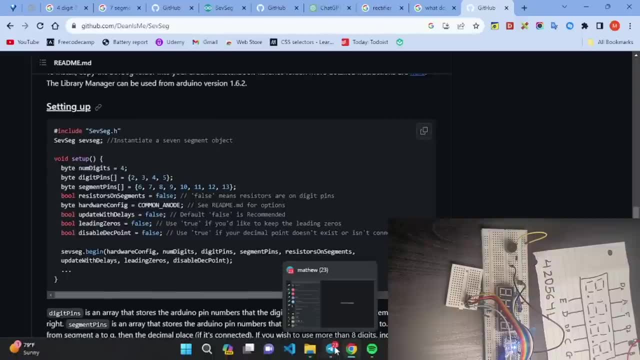 Cephseg library documentation And you can go to the GitHub right here and actually read what the Cephseg is capable of. Okay, So you can read it for yourself, But I already read the documentation myself and I'm going to be what. 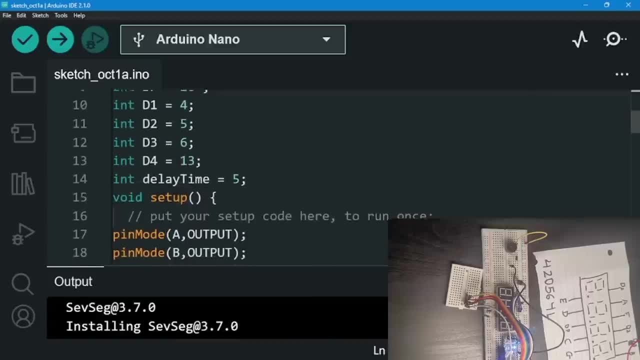 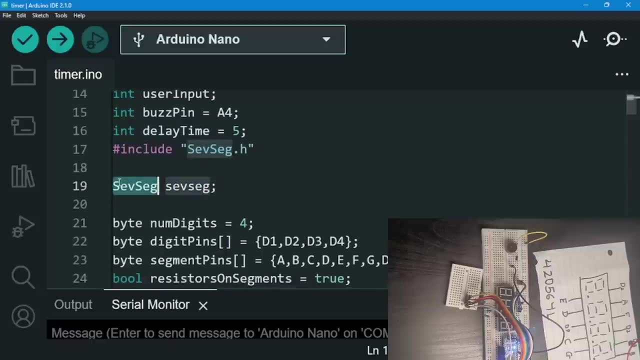 I'm just going to be using it for this purpose. All right, I just want you guys to know that. Let me just go to the. There we go. So it's basically what It's basically asking Cephseg right here, to set up an object or a list called Cephseg. 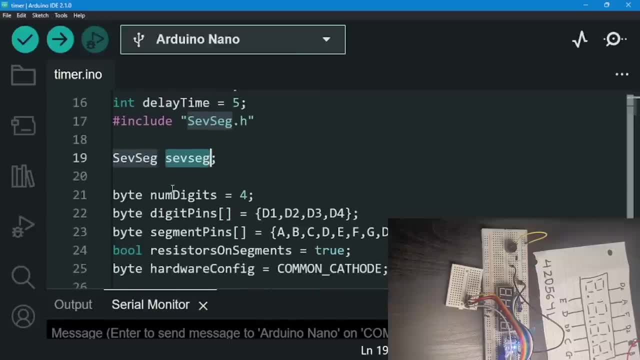 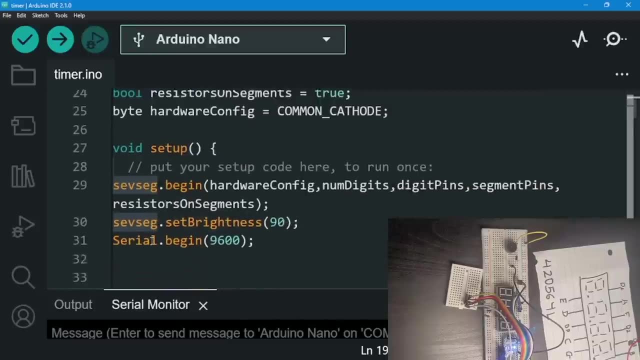 Okay, It's basically creating a Cephseg called list And we're going to be using this a lot Like. look at here I'm going to be using Cephsegbegin, Cephsegsebbrightness, Cephsegrefresh- right here, set number refresh. 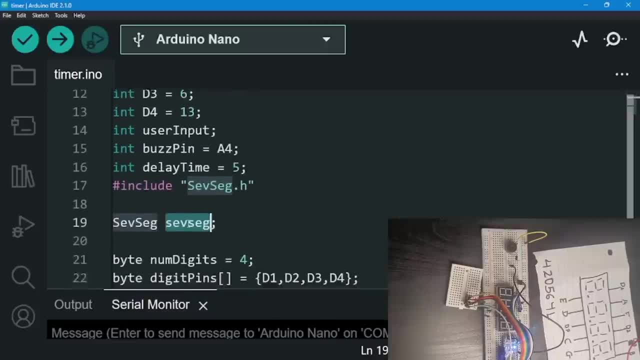 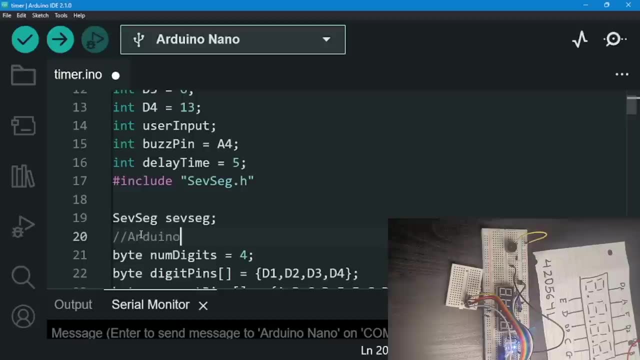 display. So basically it's going to contain the commands of what? Of the Cephseg, what Library? Okay, It's basically like how Arduino sets up. you know how Arduino is like. hey, Arduino be like. Arduino sets up what. 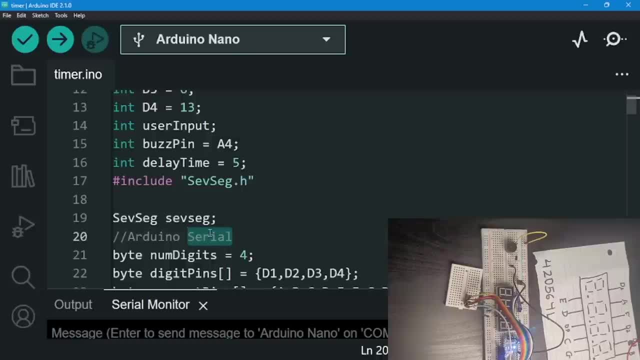 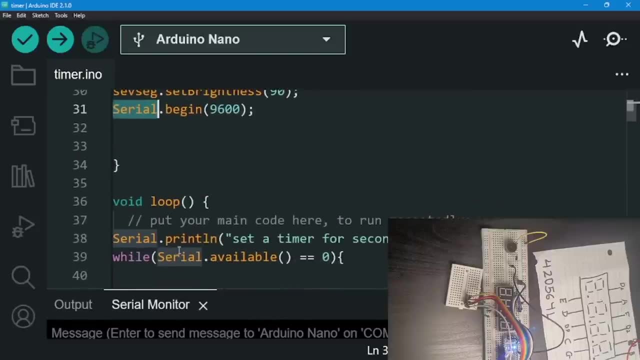 Serial monitor. Okay, It sets up an object called serial right here, A serial, Just like how we- Obviously this is automatic, by the way- It's like how we use serial and say begin, We say serialprintln, right here. 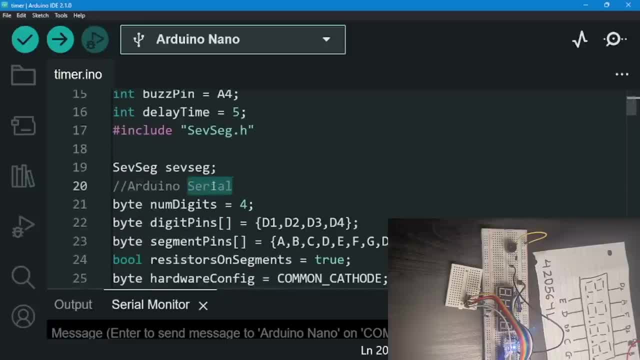 Arduino is basically what It's like. Arduino, what Setting it to what Serial? I just want you to think of it as like that equivalent. All right, But obviously Arduino does it. what Arduino does it automatically? We don't have to touch anything. 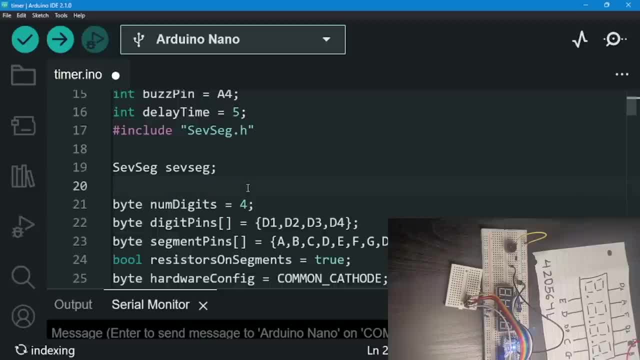 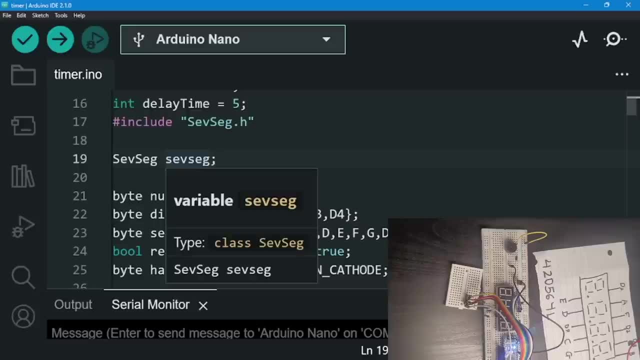 But when it comes to libraries, we have to do it ourselves. Okay, We have to do it manually. Okay, We're just setting up what Cephseg? Just think of it as a folder named Cephseg. Okay, It's a folder named Cephseg and has a lot of files. 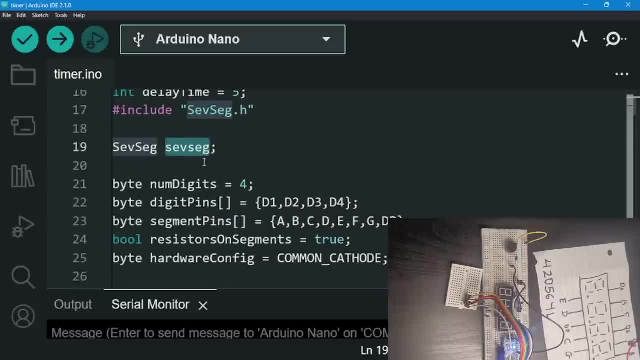 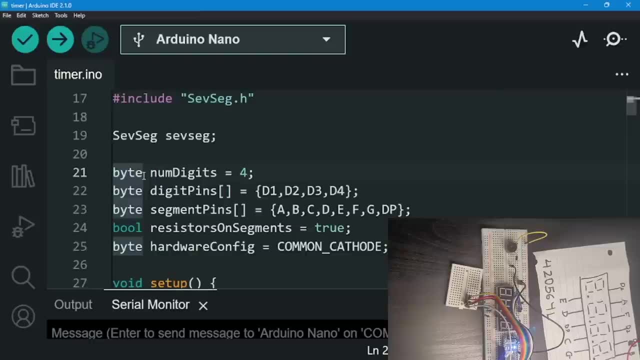 Again, okay, Lots of files right now. Okay, I just want you to think of it like that. Okay, So again, we're going to save this as a what? As a byte? Again, as you remember, we were talking about bytes. 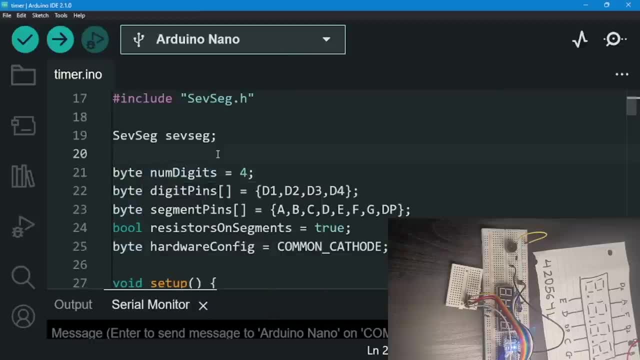 We were changing it to binary, saying 8-bit, 10-bit, and we were checking that. So basically a byte is literally what A single byte is- 8 bits, Okay. So basically it's like 8 bits of what? 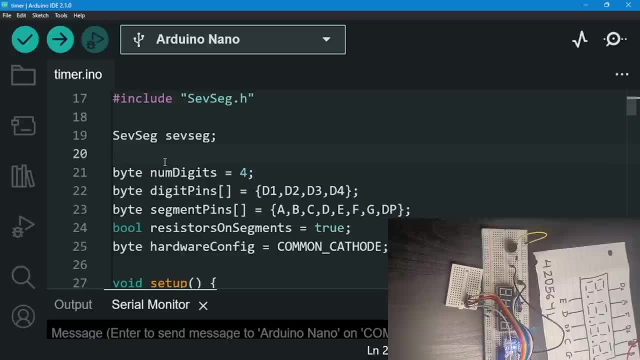 Information And we also saw how 8 bits of information literally correspond with 1 bit of information. Okay, know, when we're working with zero up to 255, for what? when we're using what? analog, again analog write command, if you remember. okay, so we're using a byte. okay, so we're going to be setting this to a. 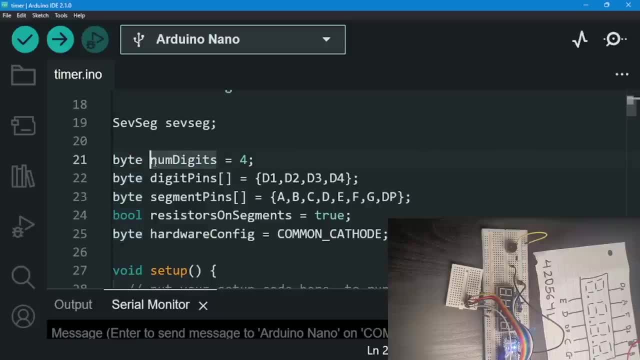 byte again. okay, and we're going to tell this and and we're going to set this: is what number of digits, basically what? for example, in our case, we have four digits. okay, we have four digits. it's gonna be corresponding to what? two, one and eight. if you go to your documentation right here, it just 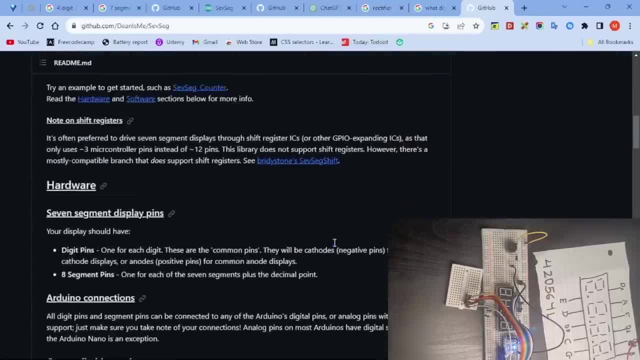 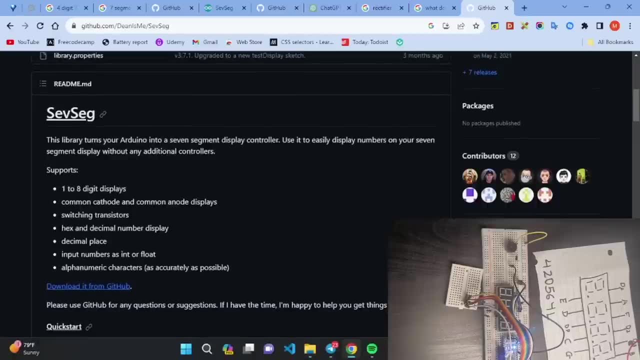 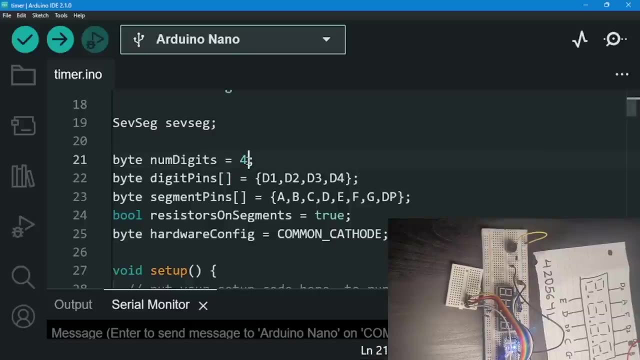 tells you right here, should be around. where is it? i actually saw there we go supports up to what? one to eight digit displays, okay, i want you to understand that. so, basically, what i did is what the number of digits that is on my one, on my seven segment led display. in this case, i'm using what? 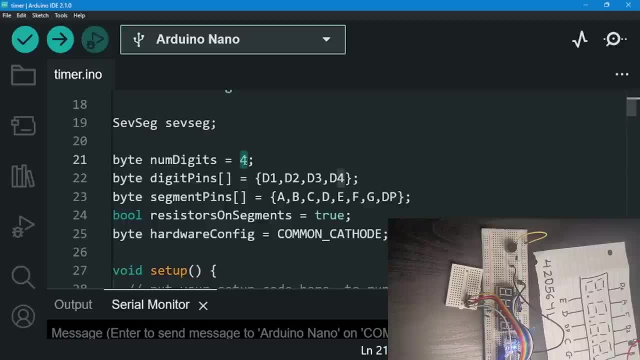 i'm using a four digit, seven segment led display. that's how i'm gonna set it up. to what? to four, and then afterwards what i'm gonna do is what? write this down again, digit pins. and then what do i do? i set it in order. okay, i say the digit pins. what are the digit pins? they're d1. i already defined them here. 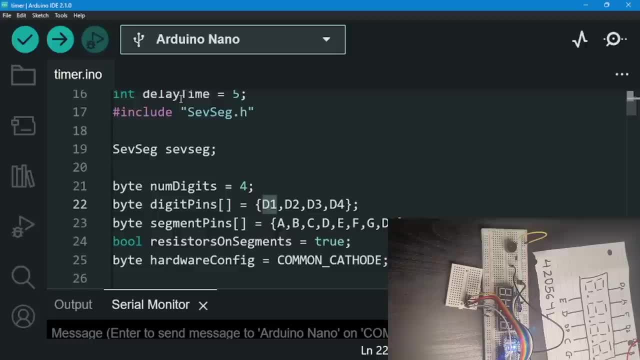 they're d1, d2, d3 and d4. okay, one thing i want you guys to understand here is: order matters. okay, you're gonna first put d1 and then you're gonna put d2 and then d3 and then d4. okay, you cannot. 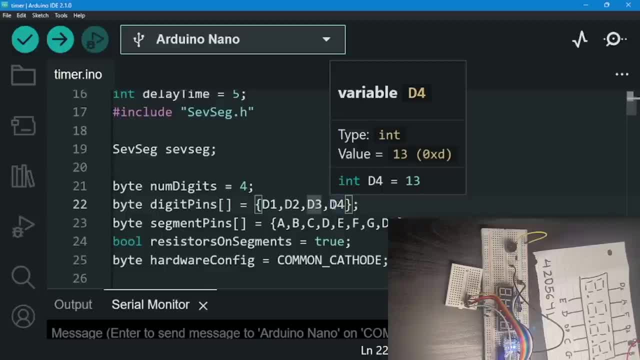 jumble it up and then expect the library to understand which one's which. okay, it's not, it's never gonna understand that. so again, one thing i want you guys to understand is what d1, d2 and d3 and d4 are supposed to be set. one and then 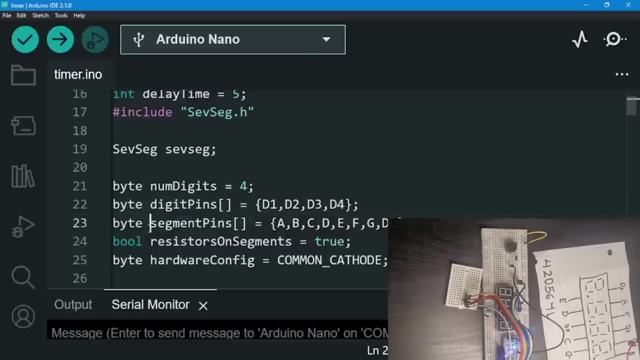 order. okay, the same goes for segments. right here, when we set segment pins. okay, it's going to be set in an order. why is that so? it's important to be in order. as i said again, there are lots and lots of models of what seven segment led displays? okay, there are lots of models of them right here, mine. 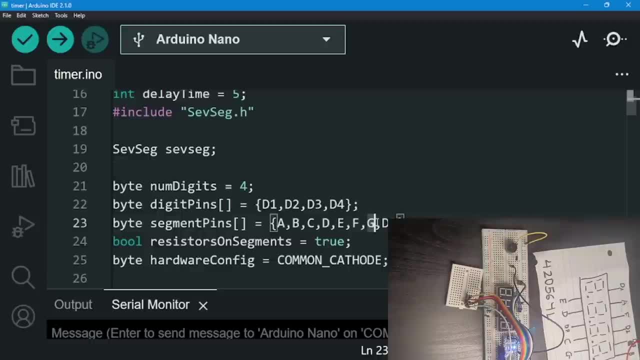 has a different number, which is 420 something, and i didn't even find the one. i didn't find the documentation regarding my type. okay, so they're going to be lots of them that are manufactured by different, again different companies. okay, they're going to be different where the pins are. 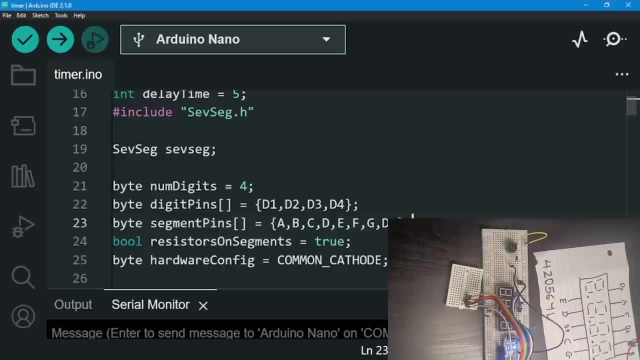 going to be what. they're going to be different from pin, from segment to segment. okay, that's why it needs to know which is which is which. okay, so you need to figure it out yourself. as i said, again, you're going to figure it out yourself and then you're going to what define it here, and then. 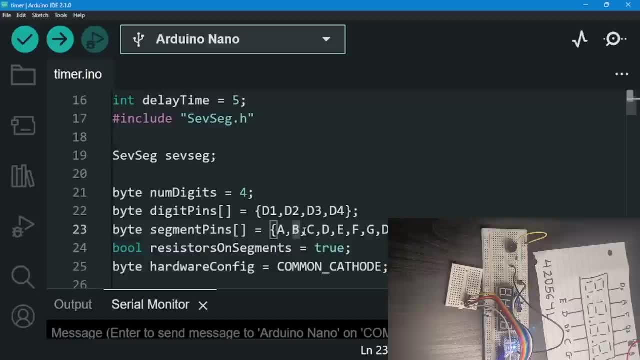 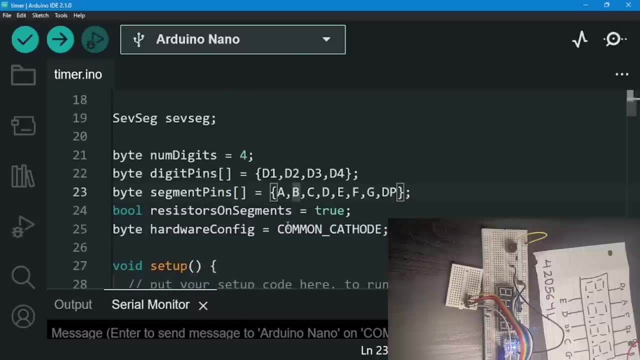 you're going to put it in an order. okay, you're going to put an order of what: a, b, c, d, e, f, g, in alphabetical order, and then finally put your decimal point. all right, then afterwards there is again, we're going to put the type of, again, the type of data we're going to store in this variable. 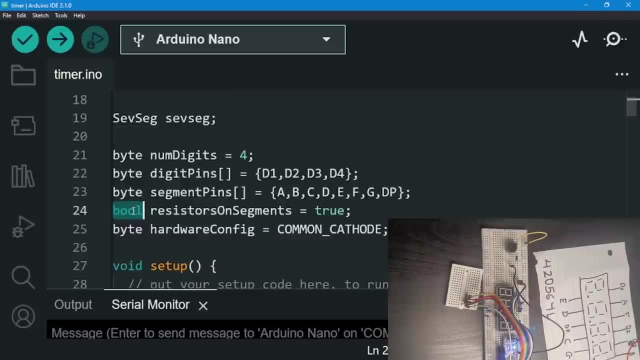 in this case it says: bull, i'm going to, i'm going to teach you guys what that means, okay. then it says: registers on segments. are we using registers on our segments? yes, we are. so we set it to true. true, basically mean what? yes, we are okay. what does a boolean mean? so a boolean, basically. 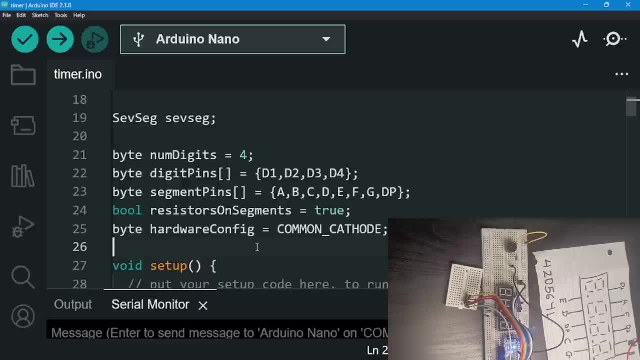 means true or false. okay, it holds two values: true or false. so true basically means i want you to think of them as being asked as a question. when you ask the question, for example, are you hungry? yes, if you're hungry, you're going to say yes, and if you're not hungry, you're going to say what? no, if 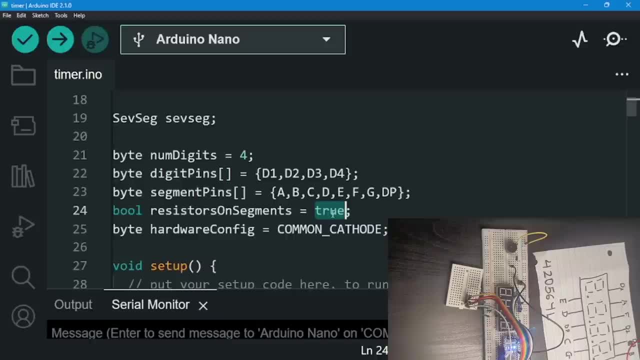 you're fully going to say what you're. you're going to say what? no, okay, that's basically it, but obviously different than what in computers. basically, you're asking our computer: do you have resistors on your segment? that's literally what cef seg is asking us, and we're setting it. 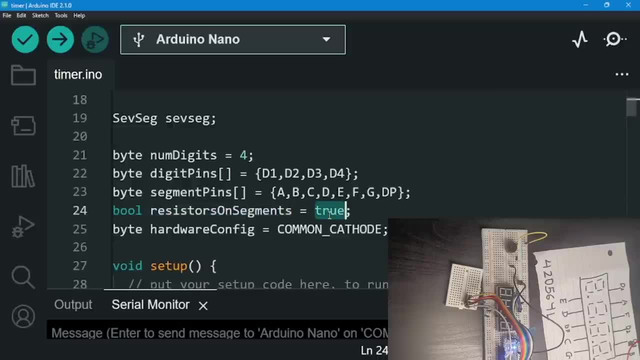 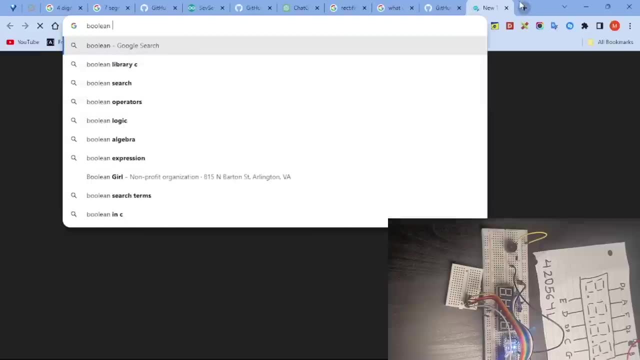 to what we're saying. yes, we do. we're setting it to what the true. okay, so this is basically booleans. okay? so even if you google it for yourselves, let's say boolean values, this is again basic computer and i think that most of you do not know, don't have prior programming. 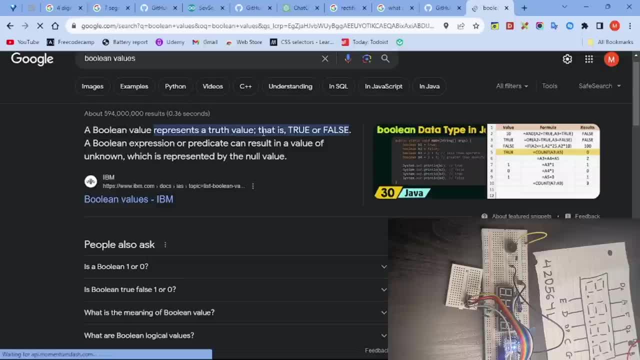 knowledge, okay, so right here- represents a truth value that is obviously true or false. okay, that's literally what it is. so, to express booleans- again they're data types, just like how we have numbers and you know strings and all that. there's something called booleans- again, they're data. 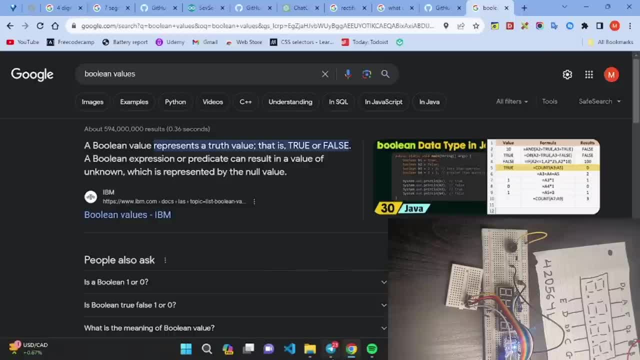 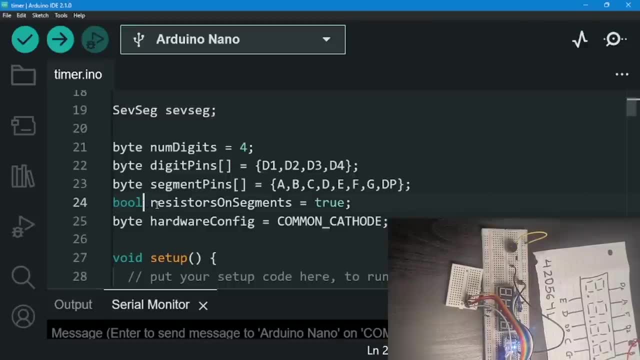 types. okay, i want you to get into detail right here. they're data types, and then we're going to represent it by what? by using the word b o o l. okay, that's one thing you should keep in mind. all right, then afterwards we tell it: the hardware configuration is yours, common cathode, or is yours? 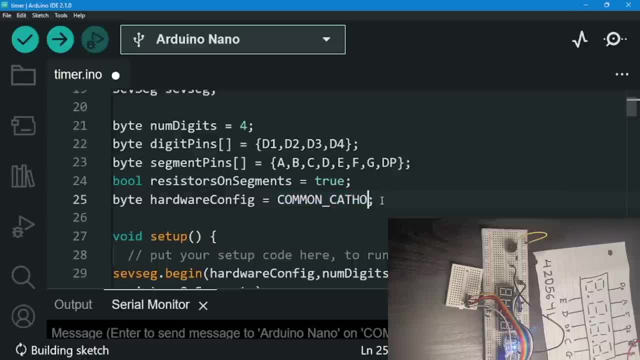 common anode. obviously, for those of you have a common anode, you're going to be what? you're going to remove this and say: common anode, there we go. it's going to finish it by itself. it has autofill, so you can just finish it by yourself. again, capitalization everywhere matters, so again, make. 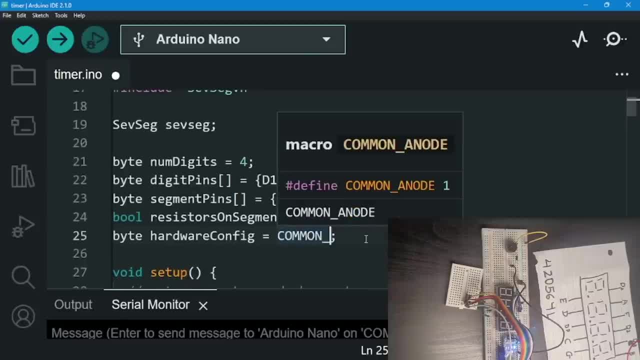 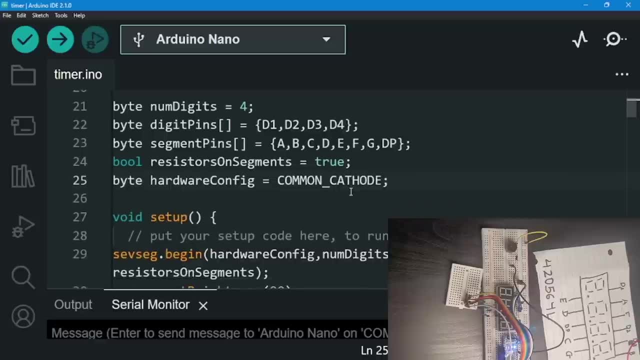 sure that you write it down in capital letters. let me just put this back to common cathode, because minus common cathode again, if you have a common annually is going to set it up to a common caveat, okay, then, as soon as what we're done, doing that, what we do is we set up our what we begin just. 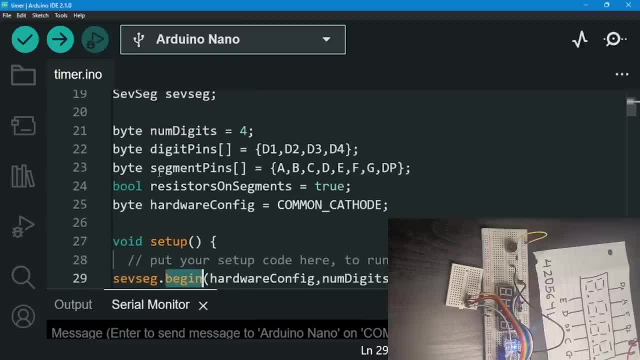 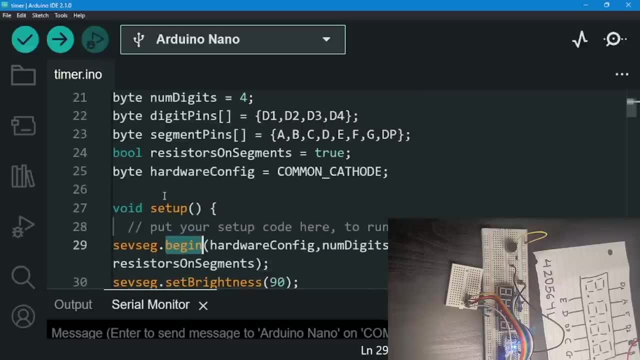 like how we begin our serial monitor. we're going to begin giving our CephSec the information. we just set it right here. what did? what did we do right here? we just set up the information and what in variables. that's all we did. right now, what are we going to do? we're going to what we're going. 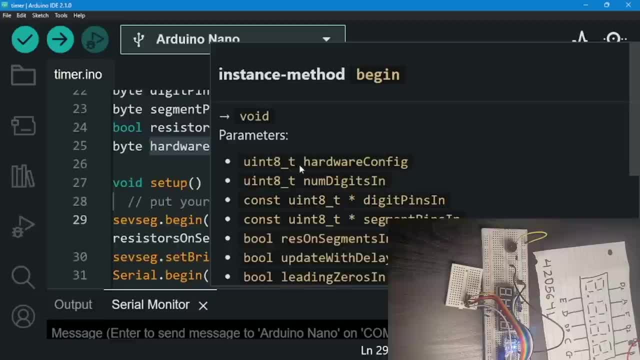 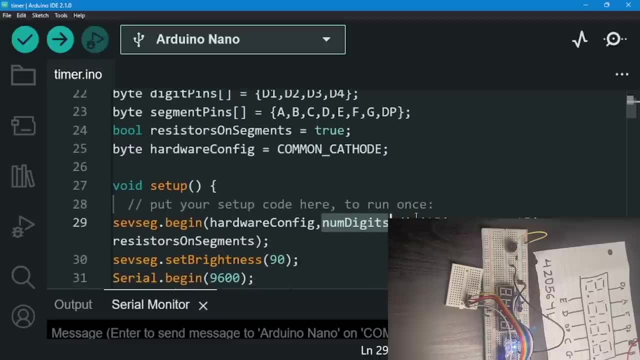 to give this information. we're going to hand it over to what? to CephSec. okay, we're going to give it its hardware configuration right here, which is going to be common cathode. we're going to give it the number of digits again, which is literally four for our case, and we're going to set our 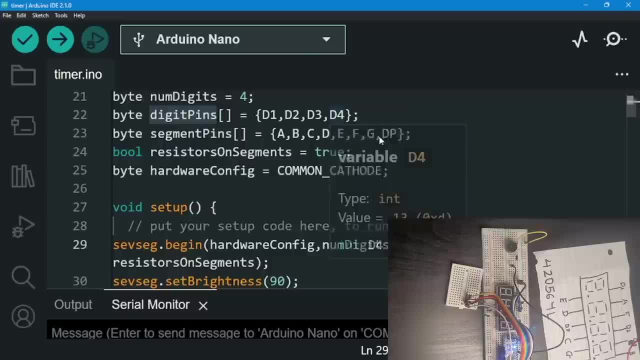 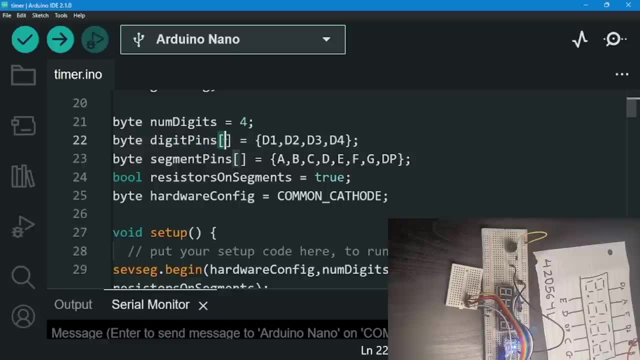 digit pins. again, we're going to give it our digit pins, the list of digit pins: right here, okay. segment pins two and then resistors on segments. one thing i want you guys to keep in mind right here is what: when we put these again squared, again squared, uh, uh, rates, right here, okay. when we put 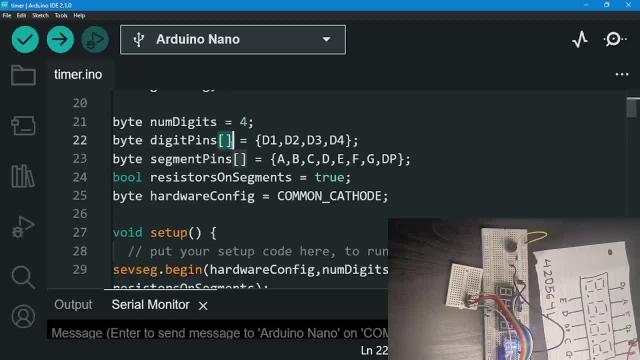 them okay. one thing i want you to understand is: we're just saying: is we have a list, okay? this means, is what? we have a list, we're going to be setting up a list, okay. so we're basically doing what. we're just setting up a list. we're setting up a list of what, a list of digit pins right here. so basically, this does what. 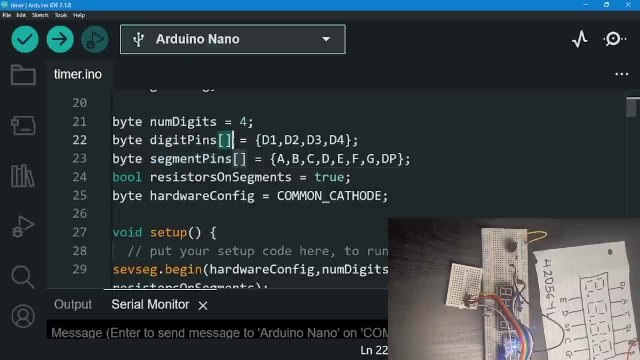 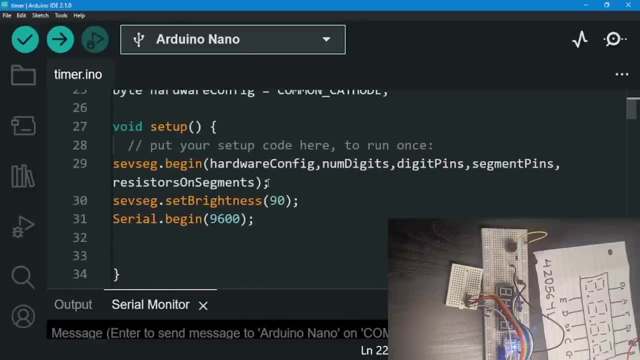 it just tells our arduino: hey, we're about to what we're about to use, list this in our code. okay, that's all it's basically telling you. okay, and afterwards, once we're done again giving this information, handing this information to sepsec, what do we do? we set the brightness right here. 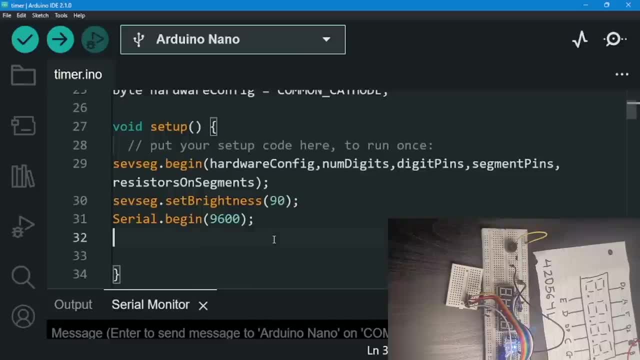 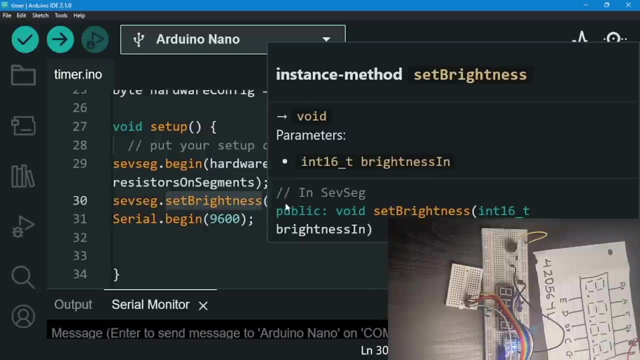 okay, and i read the documentation and it should be around zero to 200. okay, it turns it lights up from zero to 200. the value is going to be zero to 200 right here, but when it comes to 200, we're going to see something like flickering right, just like how when we're using uh, when we were using uh. 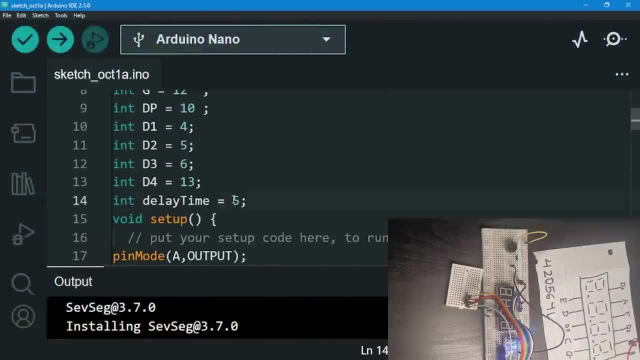 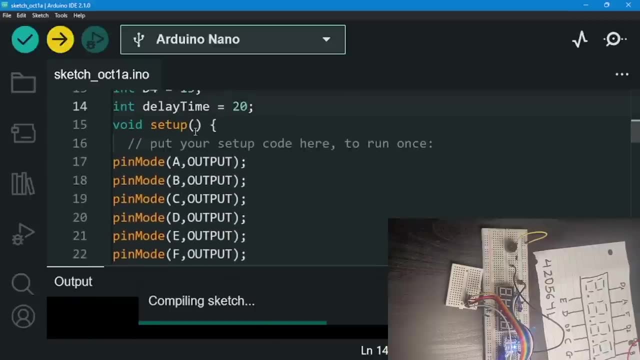 let me just bring this right here. and we set this to 20. when we set the delay time to 20, when we try to turn on everything, we see this 20 and, just like how we turn on everything, we're going to see some flickering, don't we? i'm just a compiler, just upload it. okay, i have the serial. 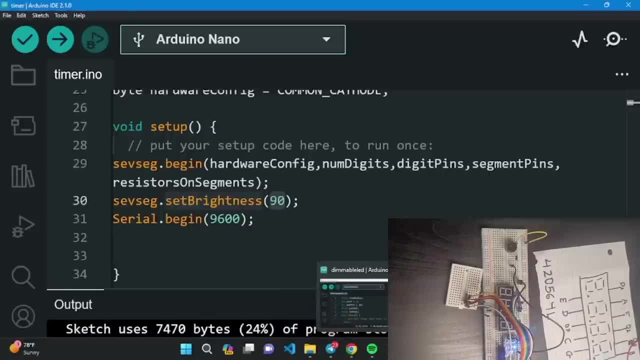 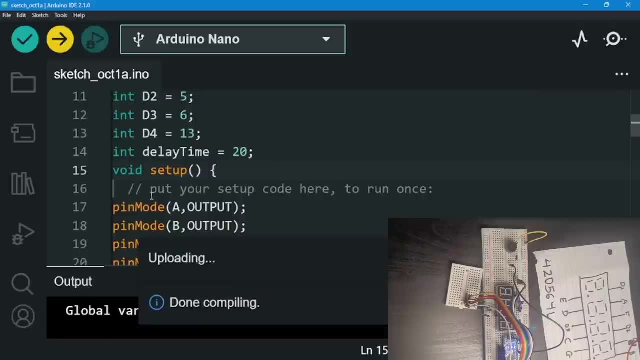 monitor open on this one. that's why there we go. now it should be working. okay, it's compiling, and now it should be uploading. it's like how, when we're trying to do that, it flickers a lot. can you see it? it's flickering a lot, can you see it? right, it flickers. 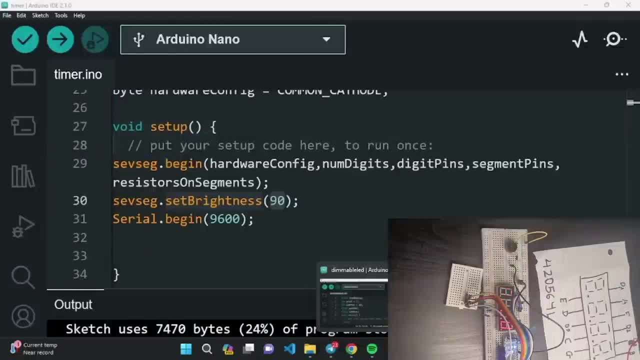 a lot. basically, that's what's happening right here. basically it's telling us right here to use a brightness between. i want you to do right here is listen, um, right here, when we set it from zero to 100, it's going to be perfectly bright, but when we set it to something above 100- for 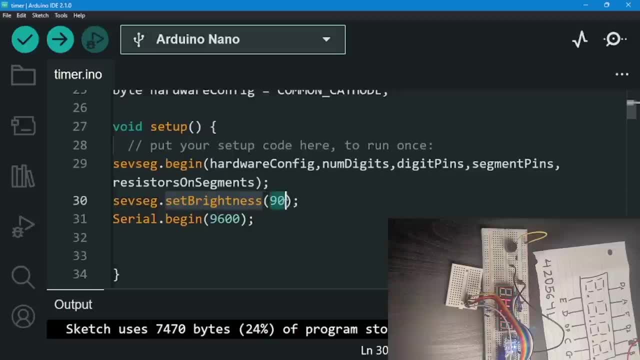 example, between 100 to 200, it's going to be perfectly bright, and when we set it to something below 100, it's going to be perfectly bright. flickering again might occur. okay, so to prevent this, i'm just going to set it to a value between zero and 100. right now, just set it to 90, you can. 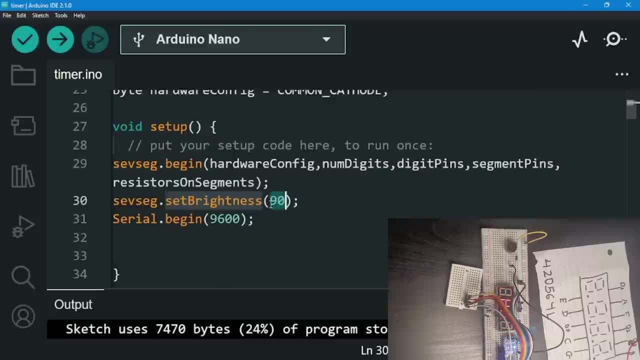 set it to 100 if you want to, but again, most cases don't use 100 to 200 value. okay, because it flickers a lot, from my experience. not only that, too, but it's also written in the documentation. okay, then afterwards we finally what? start our serial monitor right here. start our serial monitor, okay. 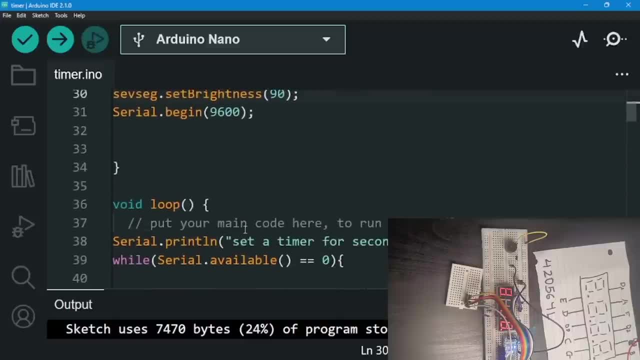 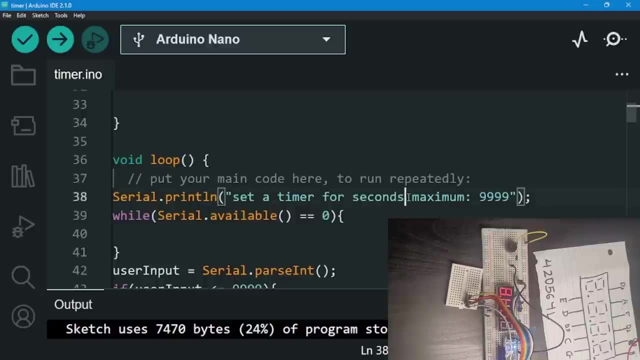 then, after we're done setting up our code right now, what do we do? now we're going to ask the user to set a timer for what? set a timer for seconds and the maximum is what let me actually set right here. should put a comma. right here makes more sense to put a comma. uh, set a timer for. 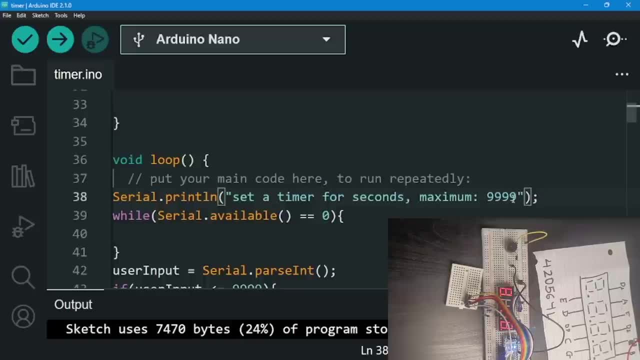 seconds. the maximum is what. the maximum is what 9999. obviously, the maximum is what 9999. i'm just saying that. okay, let's just say again, a user wants to use our again arduino and set a timer. let's just say that we're just again creating a product that is like a timer or something. 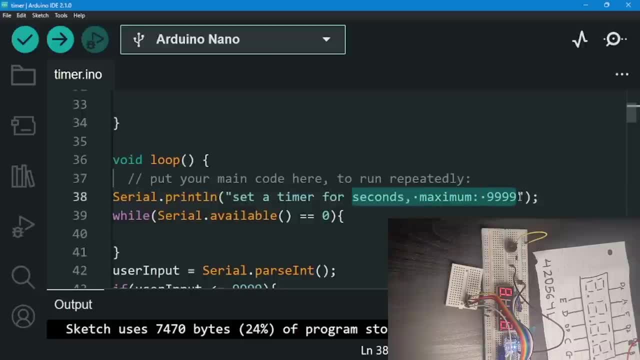 for again users, a simple digital timer. let's just say we're creating that for a user, okay, so we're going to ask it: set a timer for seconds. the maximum is what? the maximum is 9999. okay, i'm just again printing the string out and then look what happens. here there's a 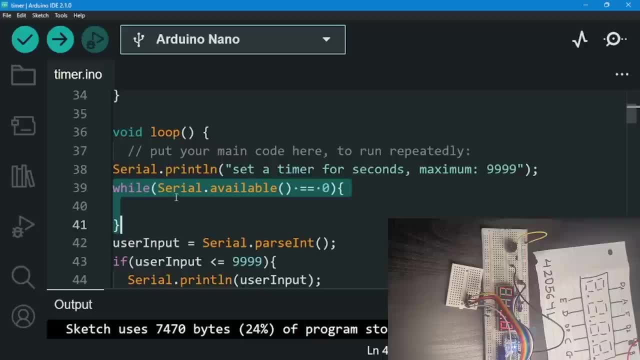 wild code right here. there's a code right here that you guys don't understand. so what i'm going to do right here, okay, just to make again our life's way simpler, let me just get out of the sketch right here and try to explain it. let me just open a new sketch and try to explain it. 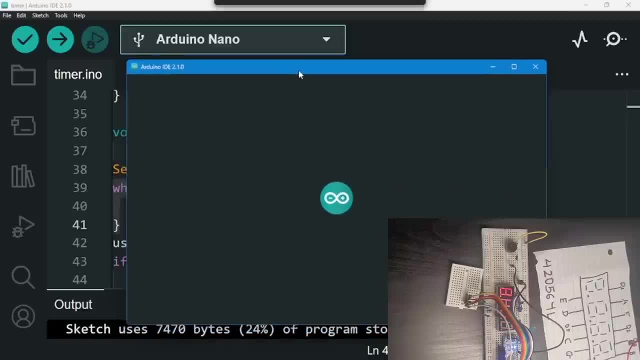 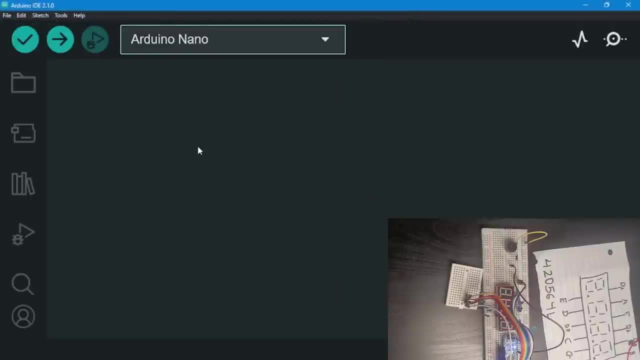 inside of a new sketch. i think it's going to make it way, way easier. let's load this load. okay, it's taking a bit. while there we go, it's loading, and let me just show you what i mean by what this loop does right here. what does even this code mean? okay, so first things first is we're going. 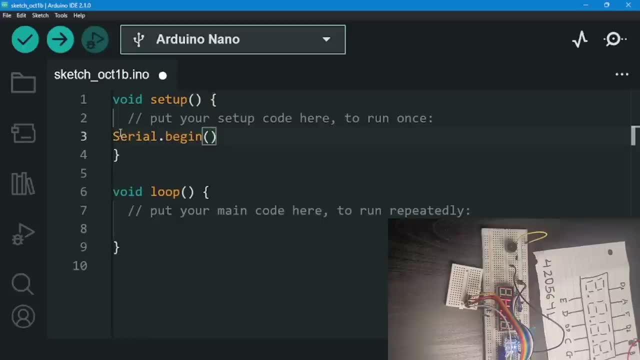 to be setting up our serial monitor. okay, serial dot begin. i just want you to follow along. i don't want you to code this. okay, i just want you to follow and just give me your attention. okay, then afterwards, what i want you to do right here is: we're going to write down while and then we go. 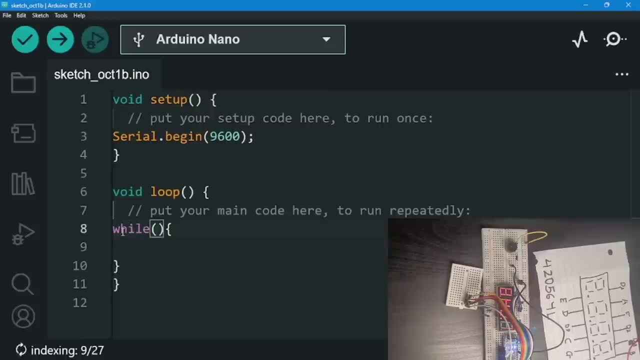 here and then, right here, set something called: we're going to be using the serial again and we're going to say available, okay, and we're going to set this to zero. we're not going to set this here, we're going to compare it to zero right here. and let me just try to explain this code for you. but before that, let 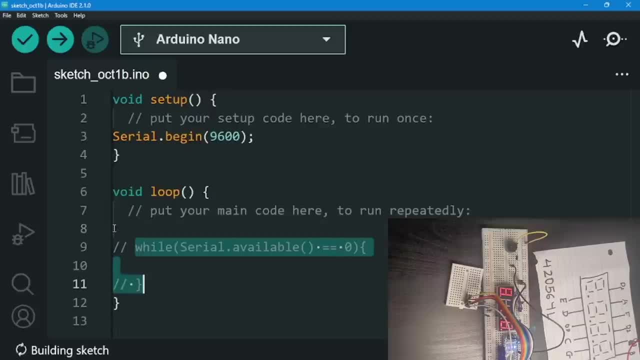 me try to print something without it, so let me just comment this out. basically, let me just leave this out for now. let me just try to print something. let's see the problem that there is and let's see the problem it solves for us. okay, let's see what this cod, what this code, solves for us. 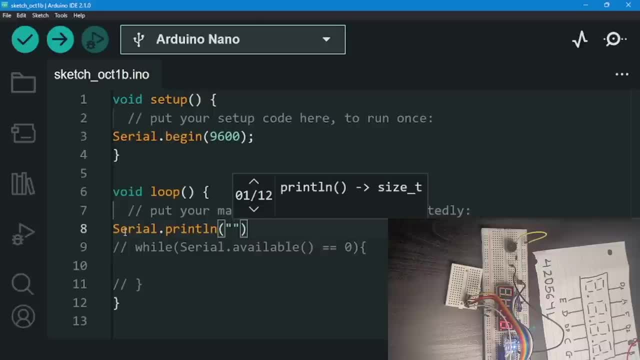 okay. so let me just again try to print what let's say. uh, let me just try to ask it a question right here. hi, how are you? okay, i'm just trying to ask it a question right here. let me set a semicolon right now and let's see what happens. okay. 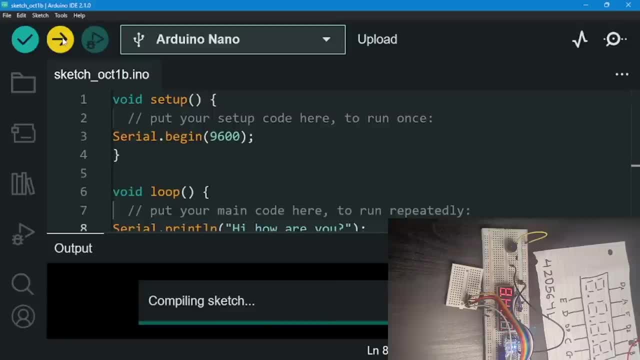 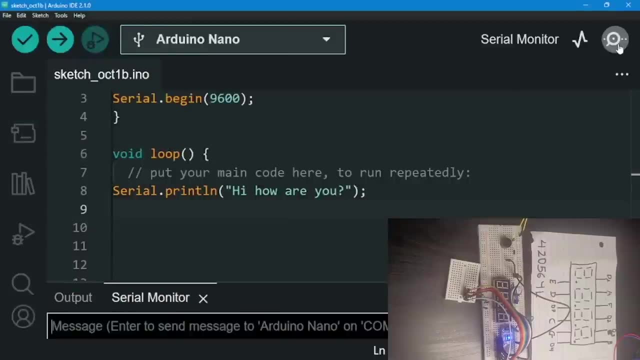 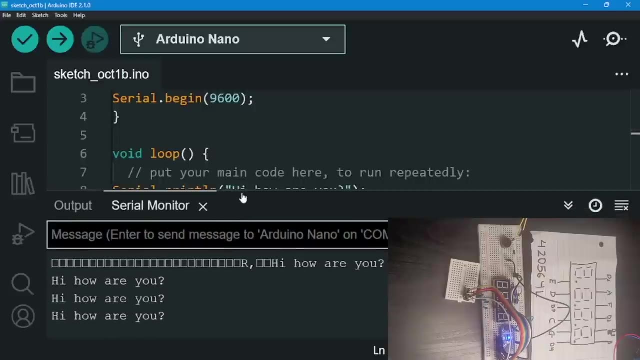 let me upload this and it should be done uploading. it's compiling and it should be done uploading by now. okay, it's done uploading, so let's see what happens here. so let me turn on the serial monitor and just go close to it. let me see that it's printing out the same thing. hi, how are you multiple? 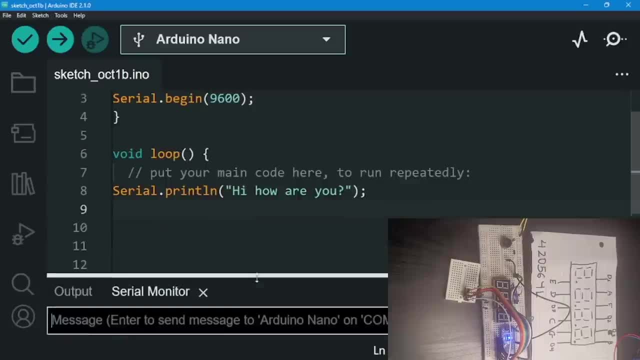 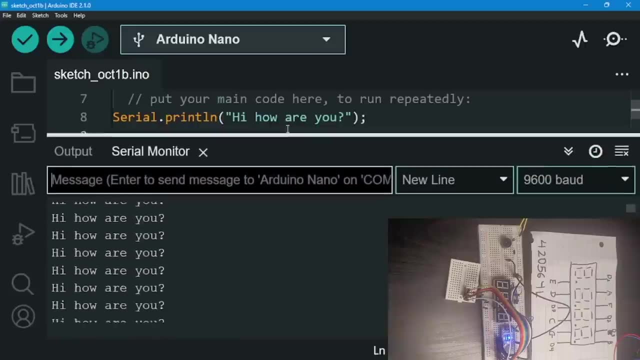 again, and again and again. can you see it? just printing it out again, infinitely. so it's just going through a loop, again, printing it, again, printing it, again, printing it. so just think of just being in a conversation and somebody asks you a question: what do you do you? what you go? 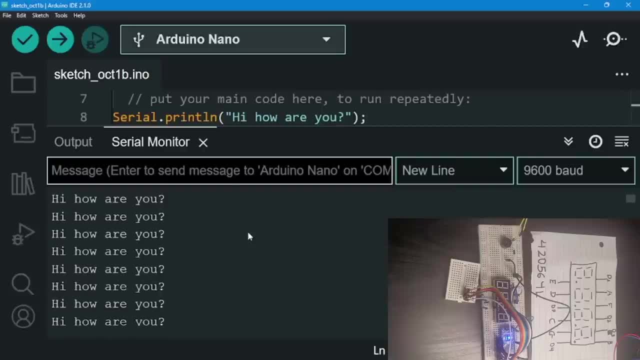 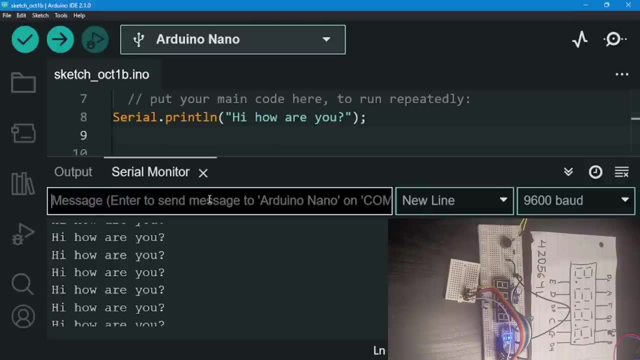 silent and what? wait for a response, don't you? you go silent and you wait for a response. basically, arduino is what arduino is: basically asking us the question over and over again, and just think of somebody doing that in real life. that would be really really awkward and really weird, really so. 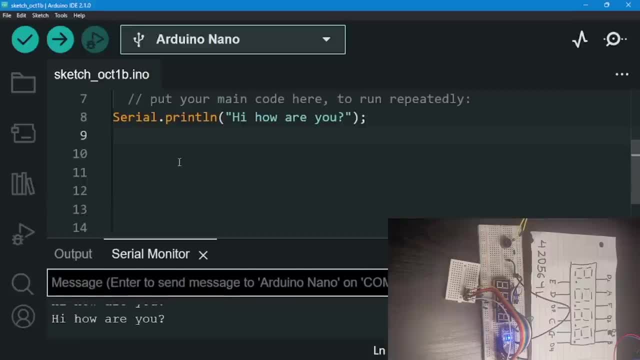 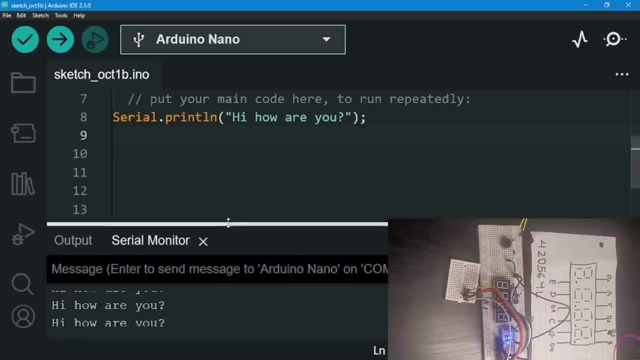 do we stop arduino, you know, from telling us, you know, from um, from again? how do we tell arduino to to again, to tell it to shut up right now. hey, arduino, i just want you to shut up until i give you a response. how do we do that? so obviously we're going to be using the wild loop right here. 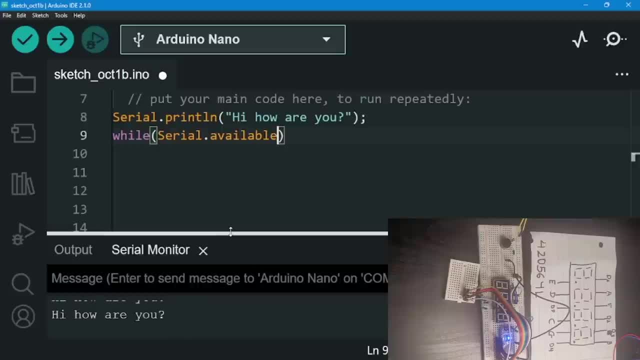 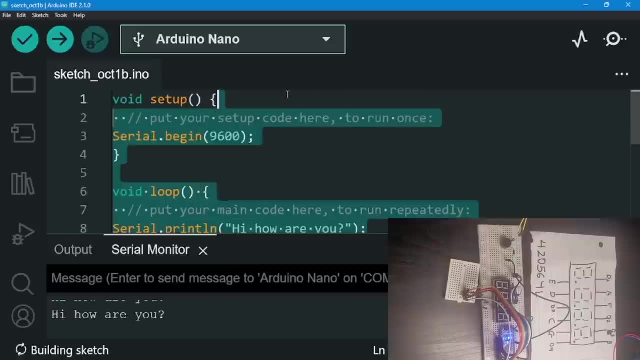 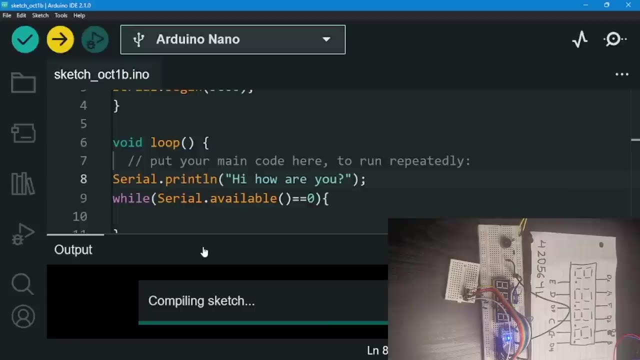 okay, and we're going to be saying: serial dot available. okay, there we go. equal to what? equal to zero. and then when we set it to here again, what does it show right here? basically, now it's going to give you a response right here. so i'm going to go this way, i'm going to go with serial monitor. 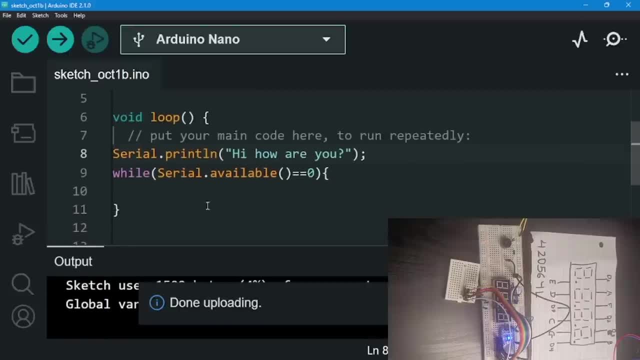 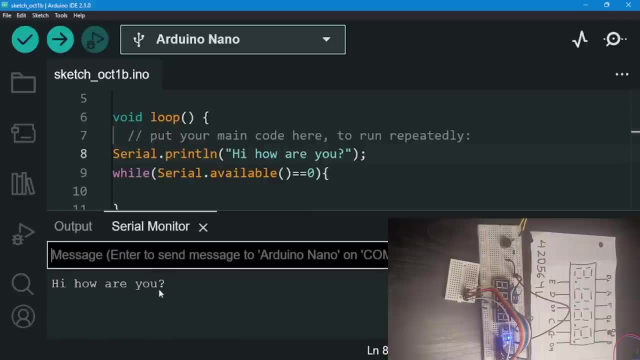 okay, so i'm going to switch to serial. and here it's going to show me that i have one time right here. okay, so i'm just going to remove the serial monitor when uploading it. there we go, ask me. it asks the same thing. there we go, still uploading. so right now, what does it do? stops asking me the. 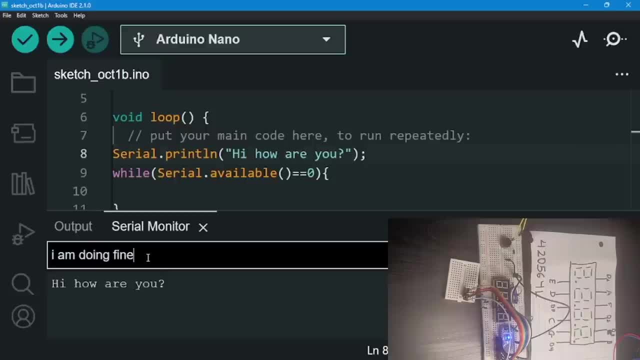 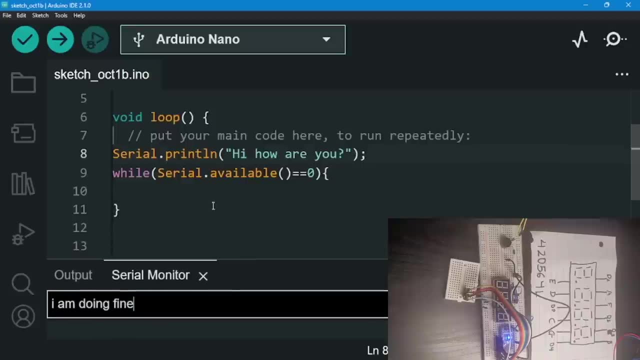 question. it just basically stops asking the question, just asks once and then waits for my response. can you see that it waits for me to enter a message right here? let's say i'm doing fine. So again, SerialAvailable checks the amount of information that is coming here through. 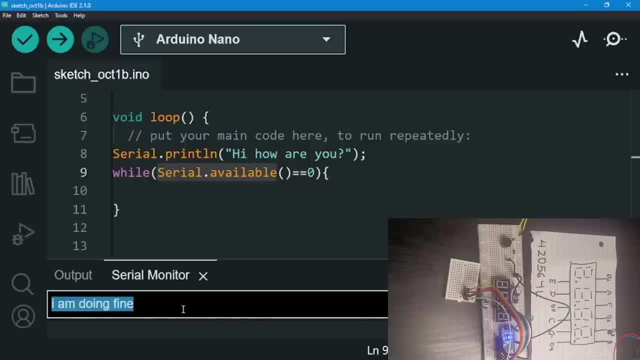 here. So, basically, the amount of information that is being sent by our serial monitor right here, In this case, if we're not sending anything, it's going to be equal to what. It's going to be equal to what. 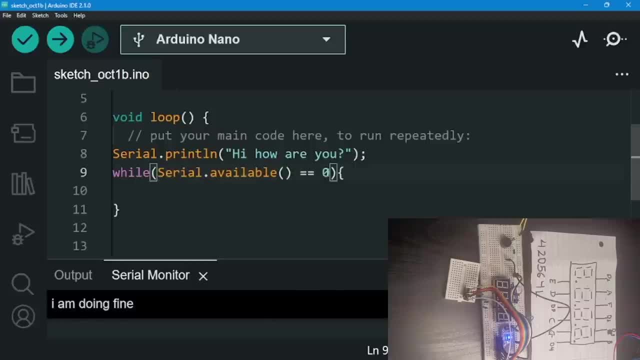 It's going to be equal to zero. If you don't send anything, it's going to be equal to zero. As soon as I send something, though, it's not going to be equal to zero right here, Let me just do that. 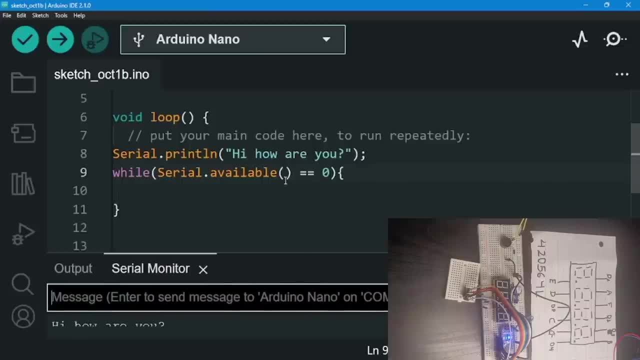 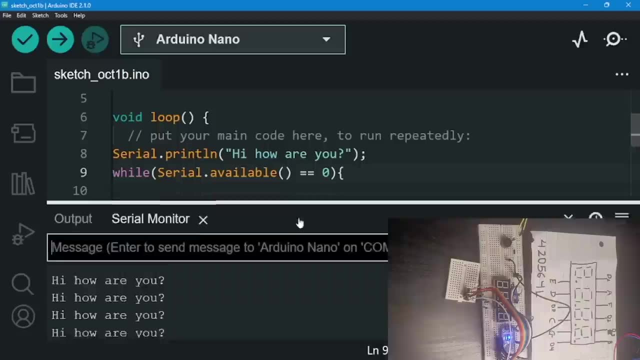 As soon as I do that, this will no longer be true. So this while loop's no longer going to be true. okay, There we go. Now. it keeps asking me the same question. Why is that so? Because it's no longer what. 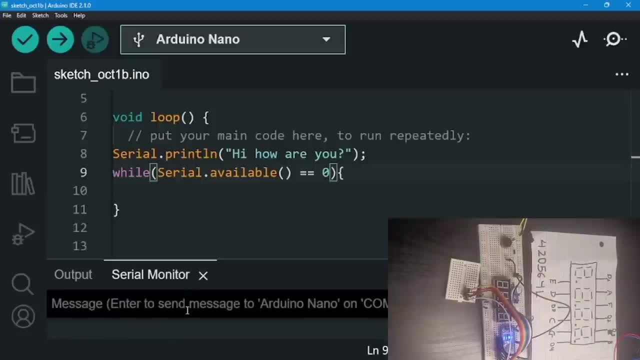 Equal to zero again. The amount of information that is being sent by the message, again by the serial monitor, is what It's, no longer to zero. I'm sending some sort of information Specifically right now. I'm sending what? 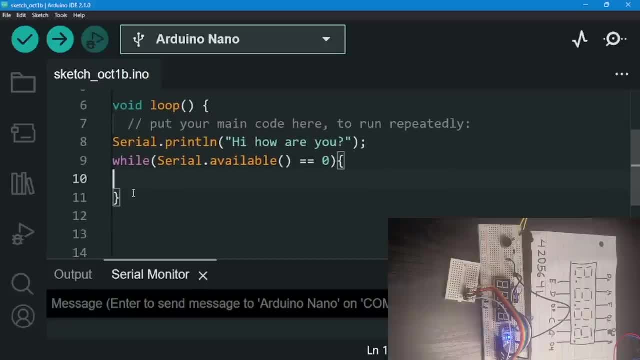 I'm sending a string, Okay, So right here. what does it do? A while loop does again. A while loop does is again. while is basically, as I said, again while hungry. we can use this metaphor again. 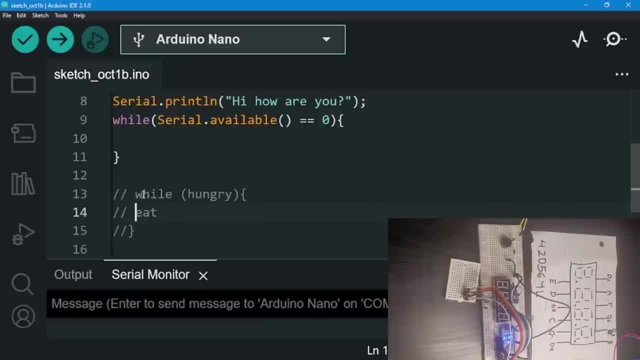 While hungry, eat, Eat, Eat. Okay, So I want you to think of them as what? While loop. I just want you to think of them as what? Again, it's going to keep on running the same thing and same thing and same thing over and. 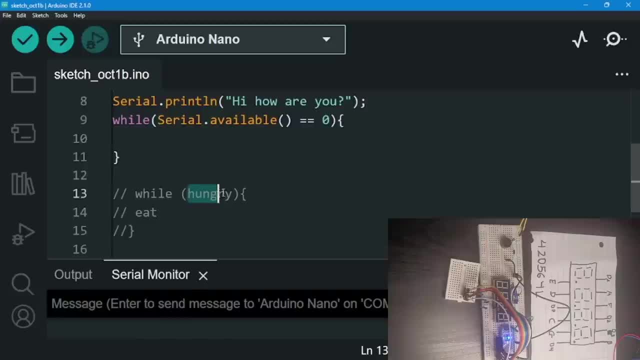 over again. until what? This condition is false. The condition that is here is what Set to false. Okay, So let's say: while we're hungry, what do we do? We keep on eating, We keep on eating, We keep on eating. 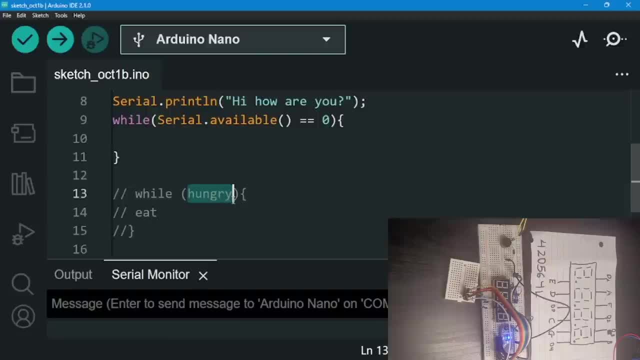 But as soon as we're no longer hungry- basically we're full- what happens? We stop eating. Okay, So we stop this. Specifically, what In this case? what does it mean? We skip the code that is in between the curly brackets. right here, the curly braces, right. 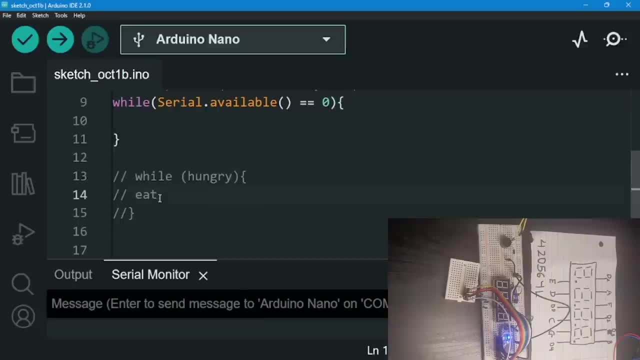 here. So we're going to be what We're going to be: skipping the code between it. Until what? Until that condition. The condition that we set here is what? It's false. So in this case, it is true until what. 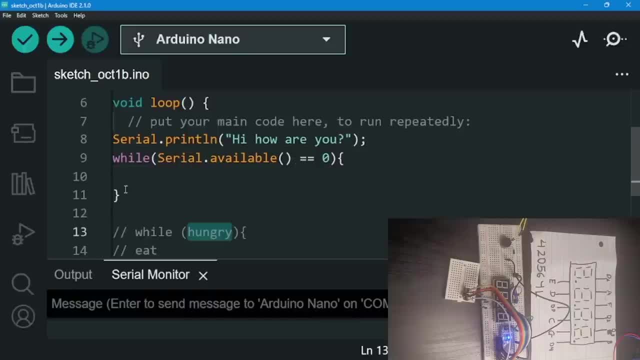 Until I give it a message right here. As soon as I give it a message, though, it's false Right here. there's nothing here. So basically, what am I telling? it is basically: wait, Wait for my response, Don't run any code. 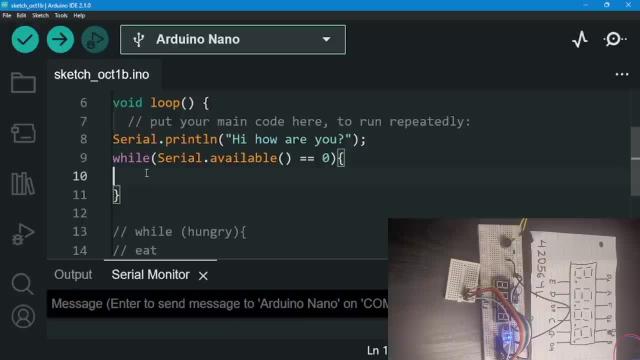 Just wait for my response. I'm just going to keep on what, Running this on a loop, on a loop, again and again and again. Waiting for what? For my response. Okay, So I was going to be waiting for my response and as soon as I respond to it, it starts. 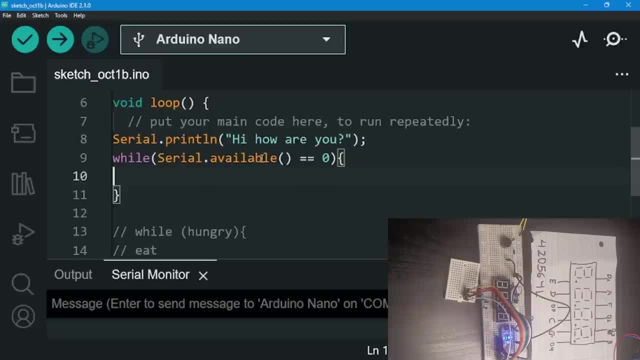 to what It starts to actually. give me what Starts to actually. what Starts to actually run the code that is below here. Okay, Starts to run the code that is found below the what, The while, again The while loop. Okay. 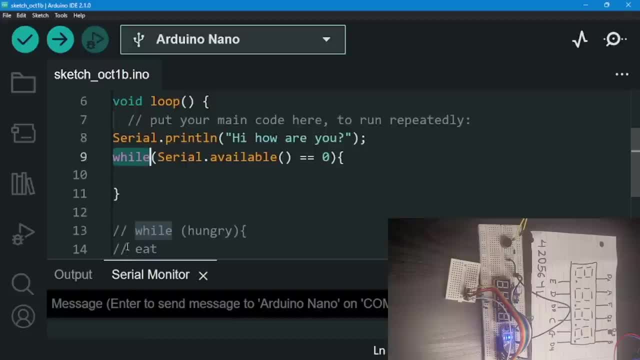 The while loop is going to keep running over and over again. It's not going to read the code that's beneath it. Okay, It's not going to be reading the code that's beneath it. What is it going to do? It's going to be reading again the while loop over and over and over again. 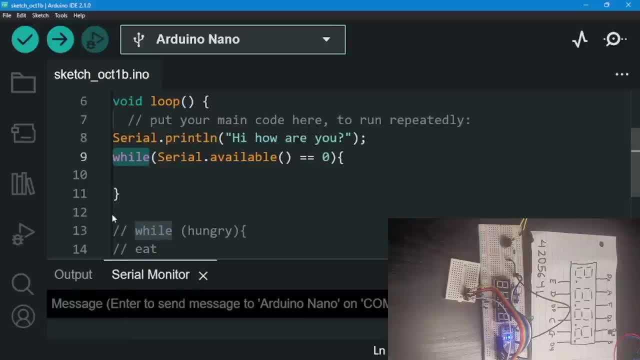 Until what? Until I get a response As soon as I do, I'm going to go beneath and read the code that I wrote down beneath the while loop. Okay, So once we just keep that in mind, let me just go to our Arduino right here. 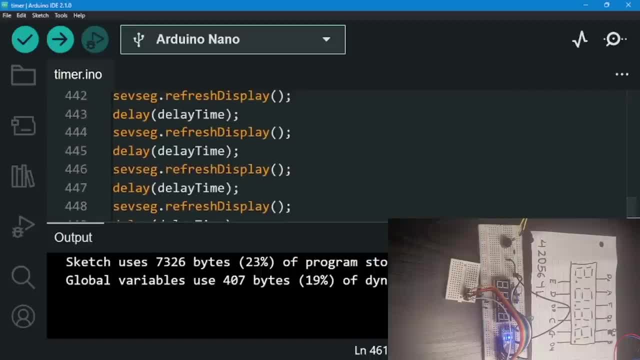 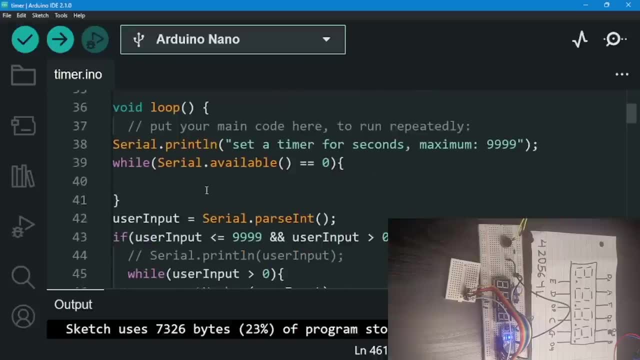 There we go. Let's go back to our actually go back to our code right here, to our while loop code. Okay, Just go here. Where is it? There we go. Okay, Afterwards, what do we do? We take the user input right here and then it's set to what. 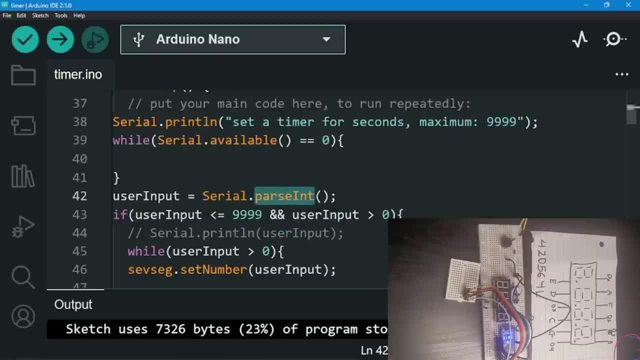 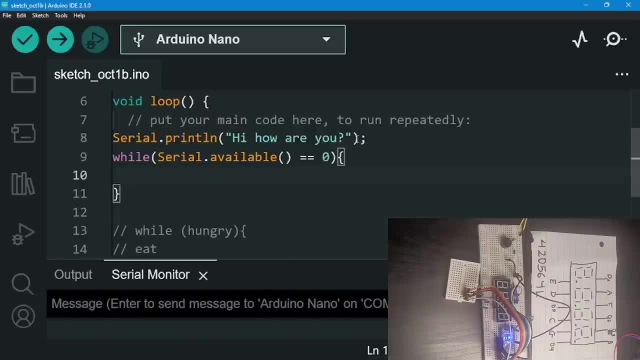 SerialparseInt. So what does serialparseInt do? So let me start from something you guys know and you guys learned about in the previous few sections. So one thing you guys learned about is what We learned about again setting up strings right here. 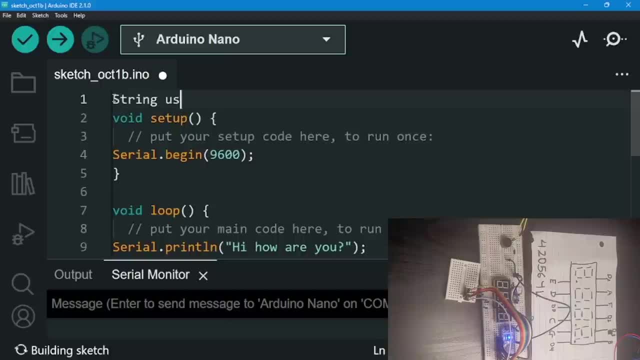 So we set up a string right here, And then what did we do? Let me just give it a name: user feed. Okay, For now Let's give it a name. Let me set it up. And then what did it do? 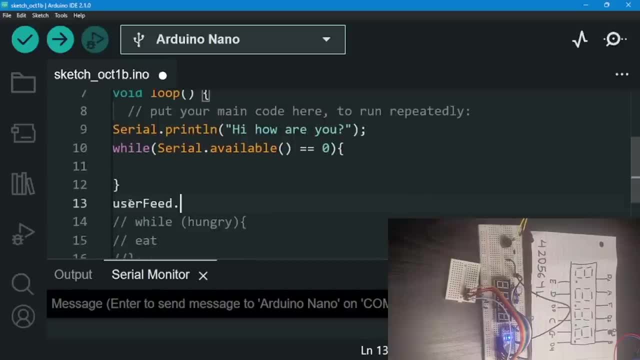 Right, here I'm going to do is I'm going to say user feed, dot. what User feed? I'm going to say user feed. I'm going to set it to. sorry, I have to set it to something. I have to set it to variable. 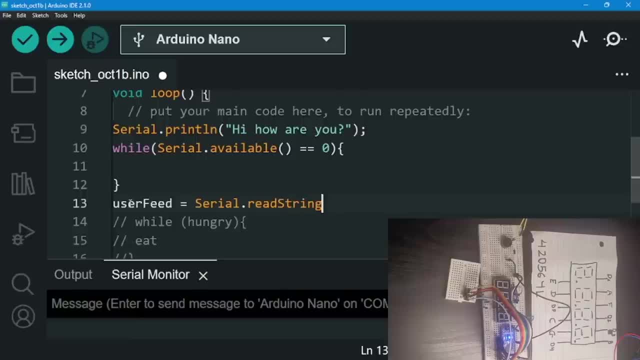 I have to set it to something. I'm going to set it to serialreadString, Right ReadString. Basically, what does this mean? Basically what It's going to read, what The value that has kind of come from here. 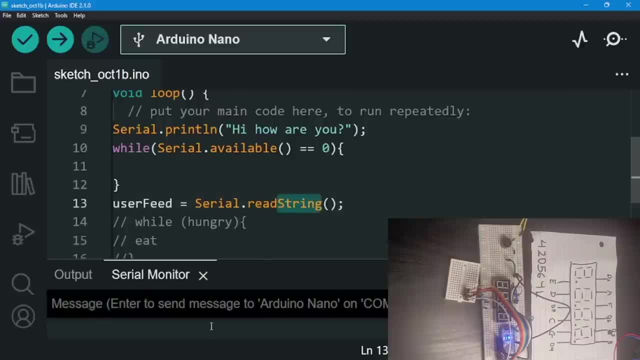 What do I expect it to be? I expect it to be what A string. It's written right here. I want it to be a string. So if I display a value right here, let me just say I am fine. to the serial monitor. 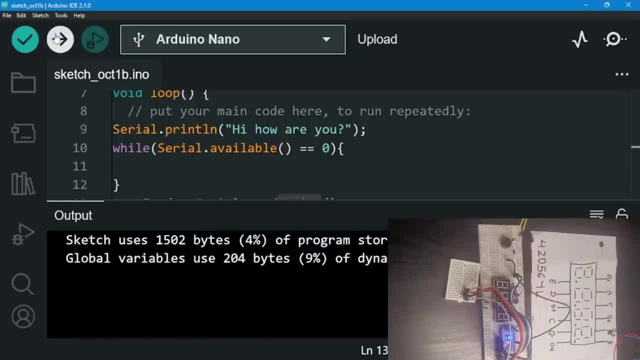 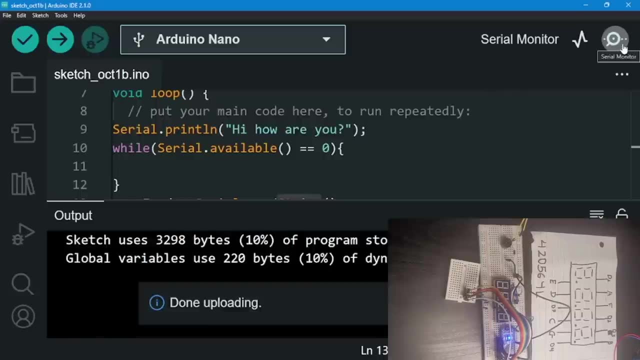 But before doing that, I have to upload it. I'll just actually upload it first. Let me upload it, And then I can just run it. Okay, It's done compiling And it's showing up. Okay, It should be uploading now. 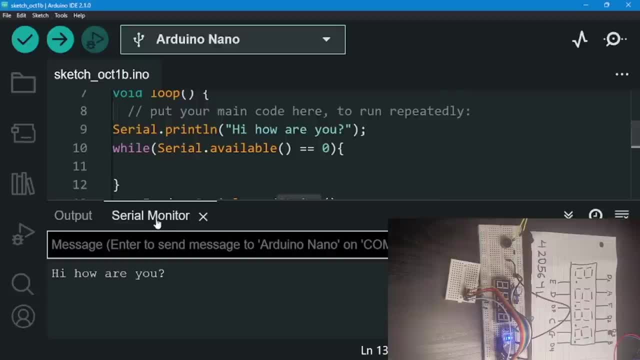 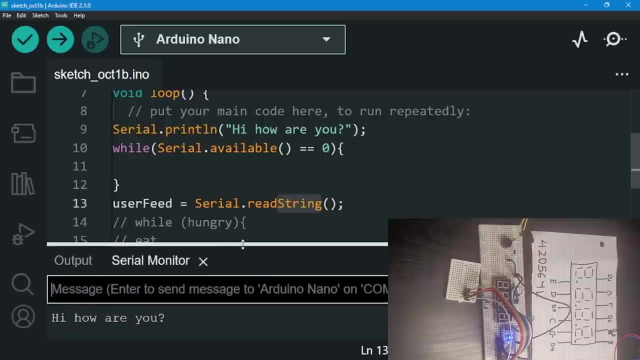 Okay, It's still uploading. There we go. Let's go to our serial monitor. There we go. And what do I say? I am fine. Okay, Let me just say I'm fine, Right here. There we go. Let me just print that user feed right now. 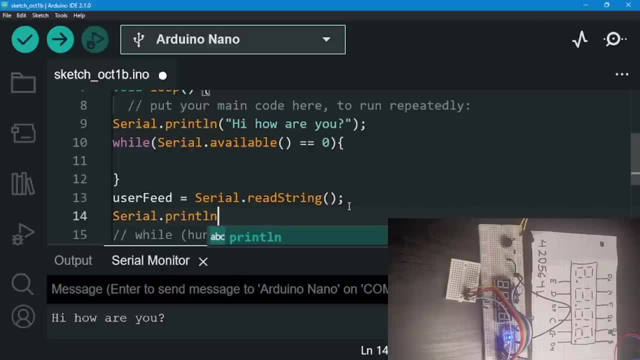 It's better to print that user feed so we can see it ourselves. Let me say println and say I want to print out the user feed. After what? After we set it up? Okay, There we go. Let me just upload it. 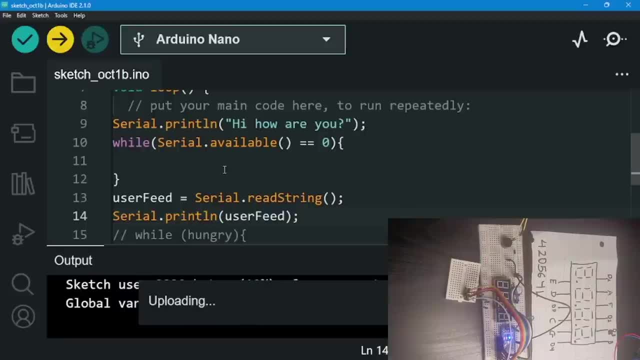 Let me close my serial monitor until that time. Okay, All right, Everything should be going good. now It's done uploading. Now let's check what happens here. Okay, Let me just say: I am fine. Okay, It prints out, I am fine. 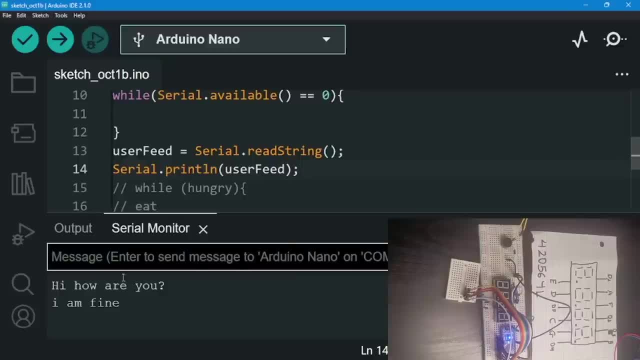 There we go. It prints out what I am fine, Nice. So what does this mean? Again? this is again used for what? For strings, Reading strings. So if you remember what did it do, It always meant what. 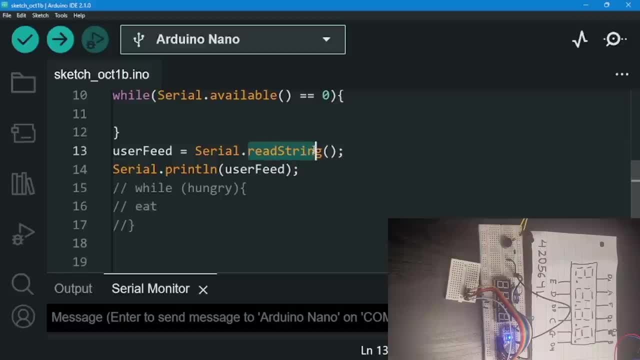 Created a new line, always At the very end. it created a new line. for what? For our responses, If you remember. Created a new line. It created a new line for what? For our responses, If you remember. Created a new line. 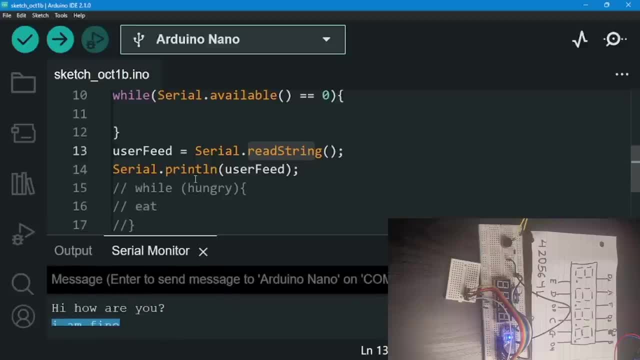 It created a new line. for what? For our responses? Created a new line, So I can just say Serialprint, And again it's going to print it out in a new line. if you remember, Now we got two. but importantly right now, what does it do? 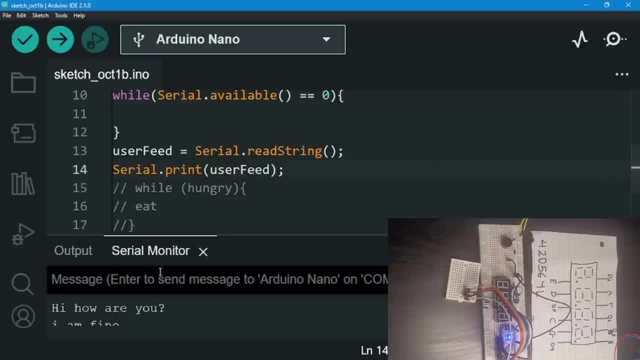 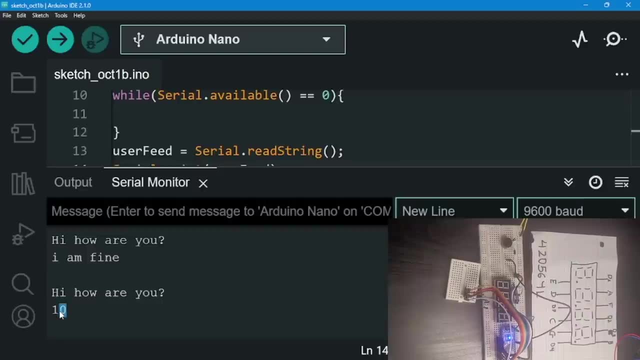 It also sets it to what, To a string. So even if I, let's say, give a value of 10 right here, if I say 10 and just enter it over here, it's going to give me what. Even though it looks the same thing, right here it seems like the same thing. 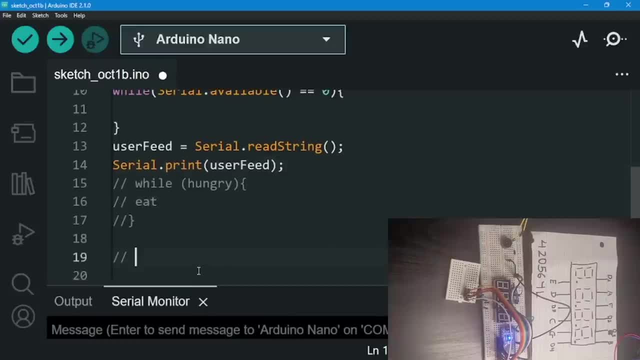 It's giving me what. It's giving me this: What Arduino is outputting is what It's outputting 10.. What I want is what, The number, 10.. It's giving me the text output, The text 10, right here. 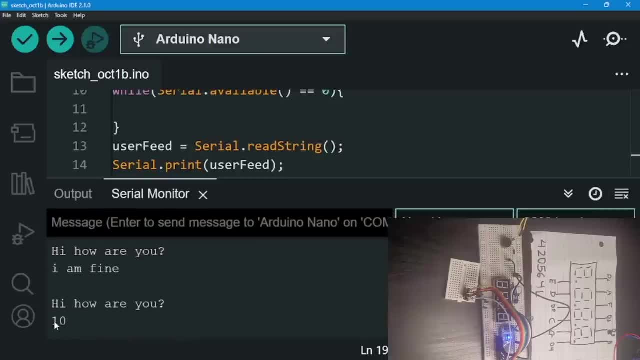 Okay, You might not see from the serial monitor. I mean from the serial monitor. you just assume that, oh, it's just 10.. No difference here. But obviously, what is it doing? It's giving me the what. 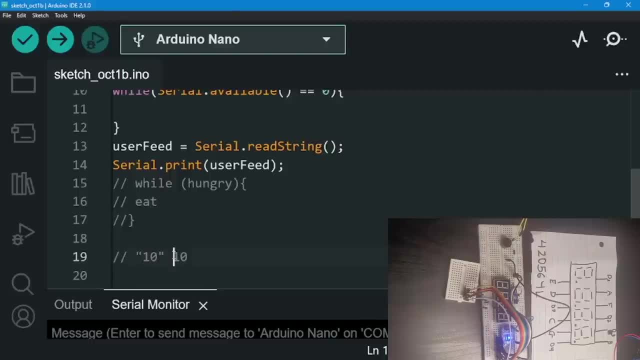 The string 10.. Okay, It's not giving you what? The number 10.. Obviously, with that case we cannot what. We cannot multiply strings, We cannot add up strings. They don't have the properties of what Numbers. 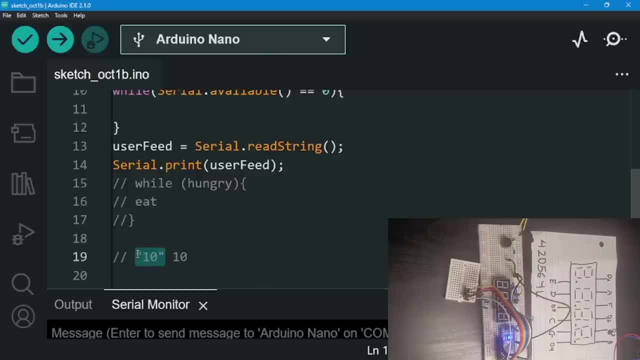 Okay, It's going to treat as a what? As a text. Arduino is going to treat our 10 as a what? As a text. when we put it inside of a string, It's going to be thinking of it as what, As a text containing what. 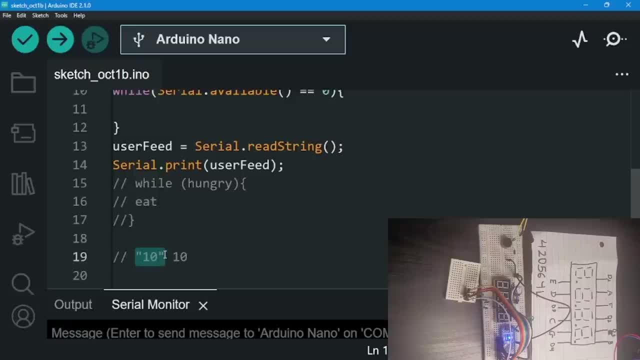 As the text, As a text containing number 10.. So it's not going to be able to multiply it, to add it, And this property is very, very important because we're going to go here. Let me just go show you guys right here. 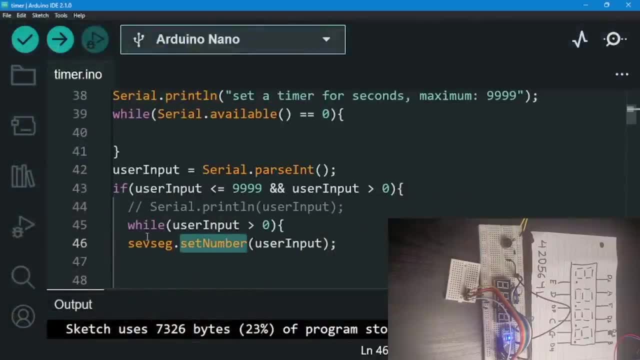 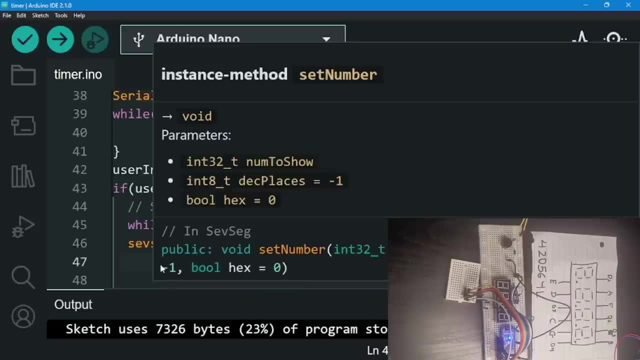 Even in our sketch right here, we're going to be using something called set number. from what? From our SEVSEG library? Okay, So we're going to be using set number. So again, when set number, obviously the name, the self-explanatory, we expect a what? 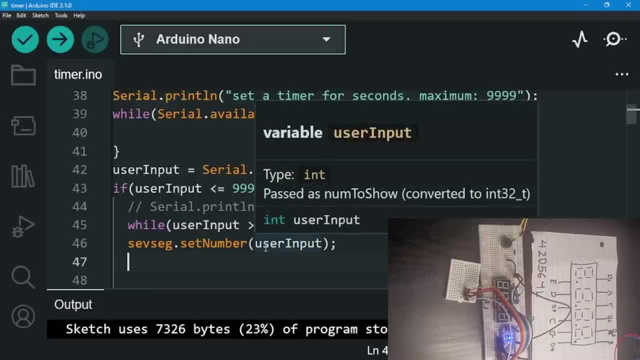 We're going to be setting a number right here. Okay, So we're going to be expecting what A number? If you put a string right here, we're going to be what? We're going to be confusing our SEVSEG. what? 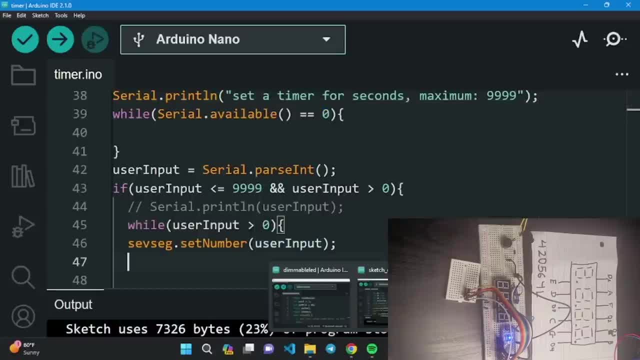 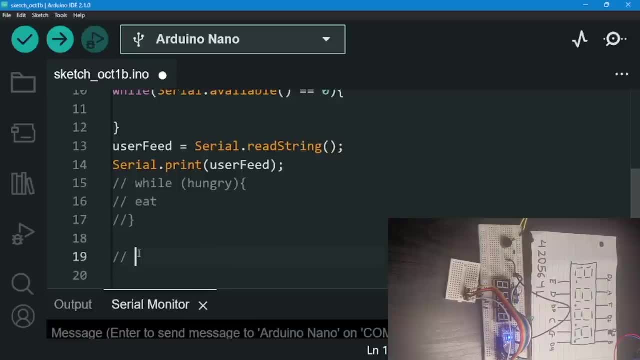 Library, Library. Okay, We're going to be getting a bunch of errors, Okay. So right here, just to make sure that we're receiving number 10, and we want to even give out numbers. is how do we tell Arduino that we're going to give it numbers instead of? 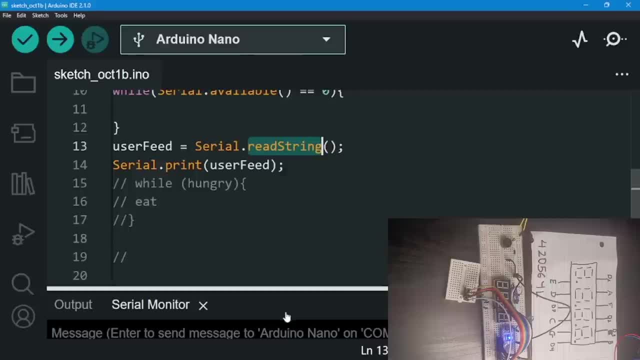 strings. How are we going to tell it that we're going to be giving it numbers is literally using parse int. Okay, Parse int. It contains the what, The name int, The integers. Int keeps what Integers. Okay, So we're telling Arduino what. 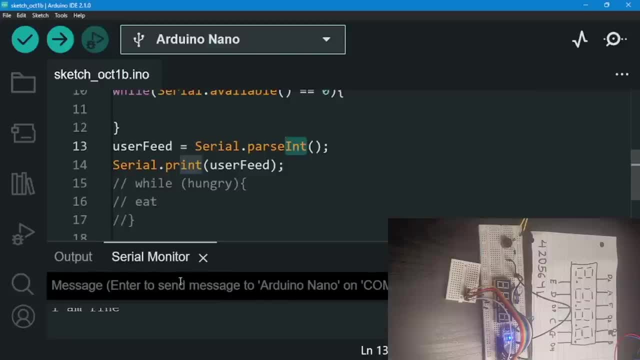 We're going to be giving it integers. Okay, In the message board, we're going to be giving it what. We're going to be giving it integers And, most importantly, I want you to store it as what. I want you to store it in the variable as a what. 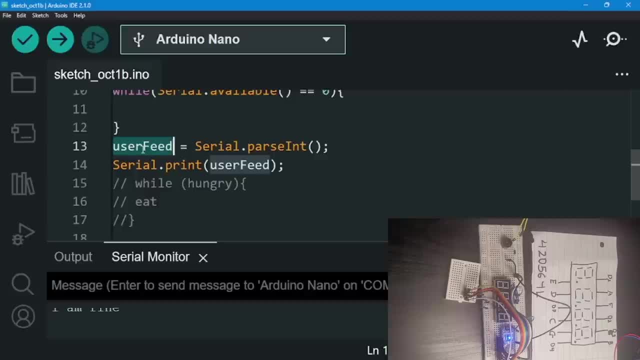 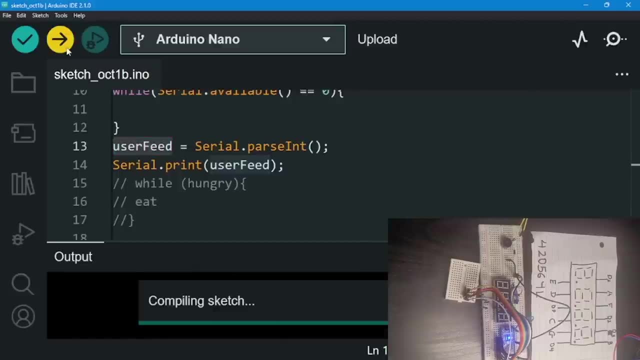 As an integer. I want you to store it as a string. I want you to store it as what. I want you to store it as a number. Okay, That's what we're telling Arduino. So it expects a number. Now, it doesn't expect a number, but also what? 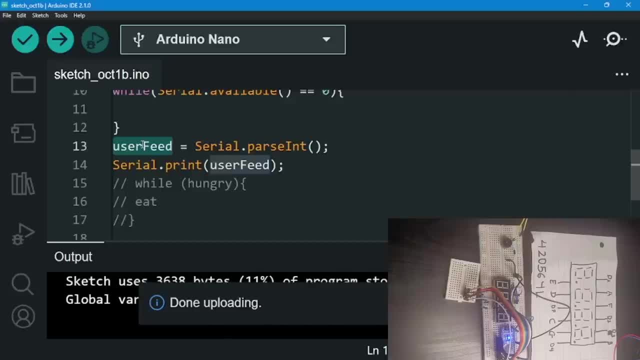 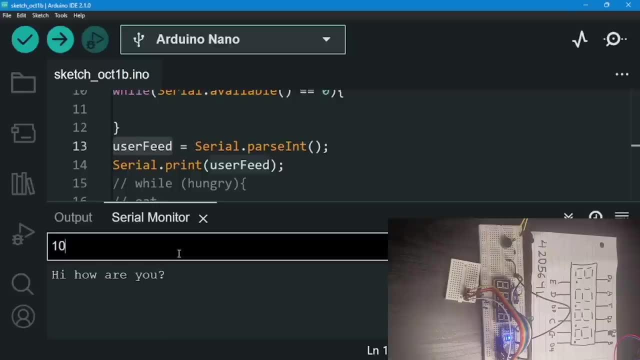 It also is going to be outputting it, And again it's setting our variable to a what, To a number. Okay, So right here, let me just say right here, and parse int. I'm just going to say 10, right here. 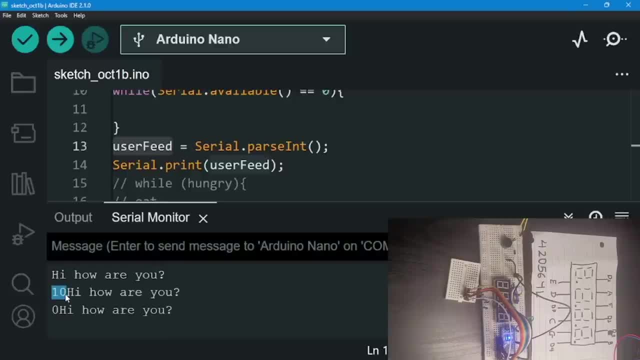 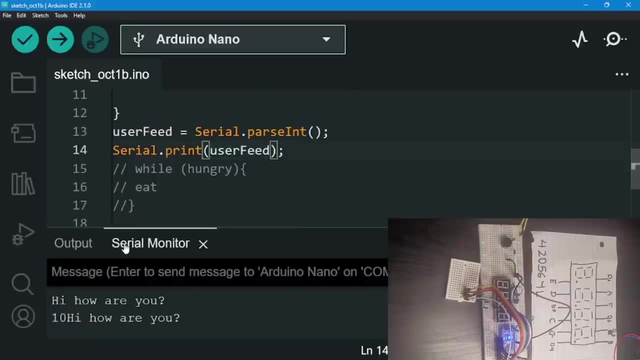 And then it's going to give me. Can you see it? I just gave it 10 right here. It just gave me 10.. Obviously, I just said print right here and not print ln. I said print right here, So it just gave me 10 and then asked the question again because obviously what? 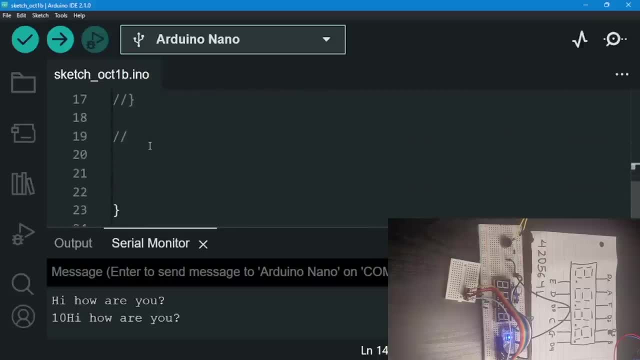 Because, again, it's running on a loop, So it's going to be asking me the same question once it's done going through the loop. Okay, So the main important thing here is what. When it comes to parse int, it's what? 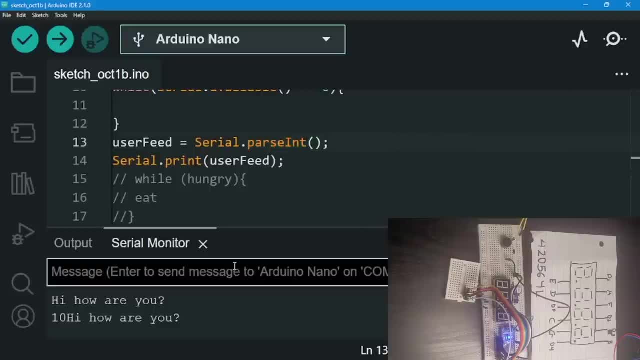 We're going to be receiving integers on the message. That's where we're telling what Arduino. Okay, So we're going to be telling Arduino. we're going to be receiving 10, not only that two, but what We're going to store it at what. 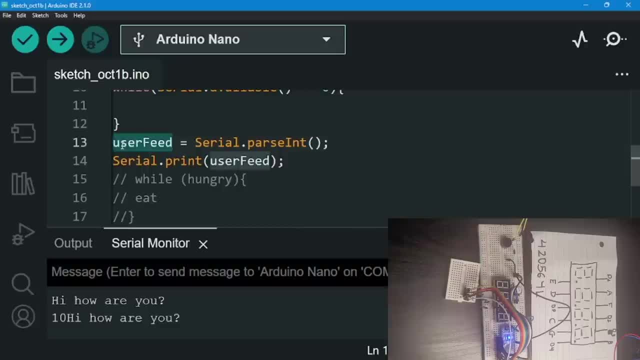 As a number. I want it specifically stored as what? As a number. I don't want you to store it as a string. That's where we're telling Arduino. Well, obviously, there's something called parse int and there's something else called parse. 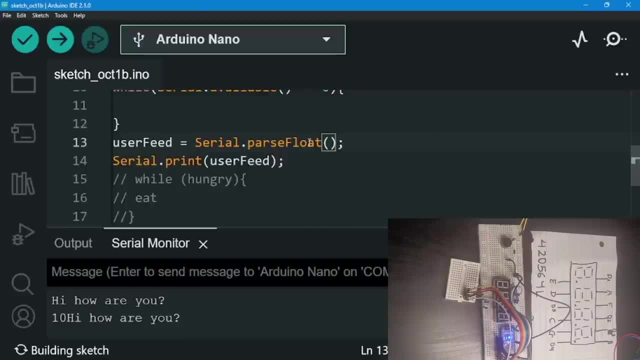 float. Basically, parse float is literally the same thing as parse int, except for what? As for float numbers, Basically what Decimals? Okay, So let me just go back to parse int. That's one thing I want you guys to know. 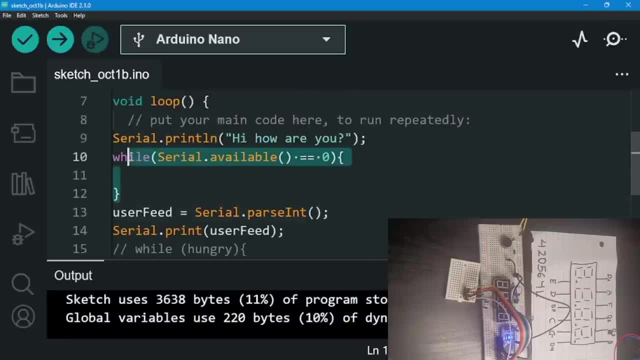 Okay, So even actually we said that we use the while serialavailable. again this loop, right here we use it again. to what? For Arduino? not to ask us the same question, but it's actually important to in another aspect. Okay, Let me just remove the question right now. 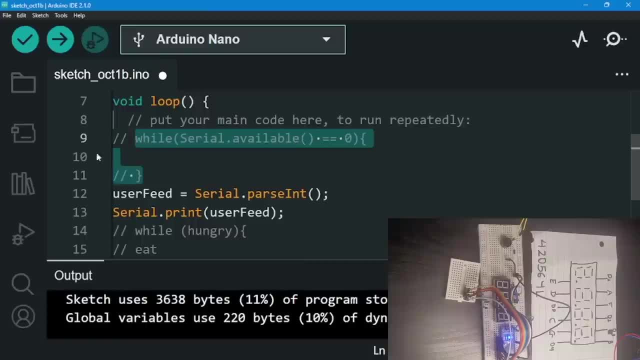 Again. let me just show you why it's important too. Just go right here. Let me just dice it out again. Let me just take it out right now and let's see, let me just upload it. Let me just try to set up a variable right here. 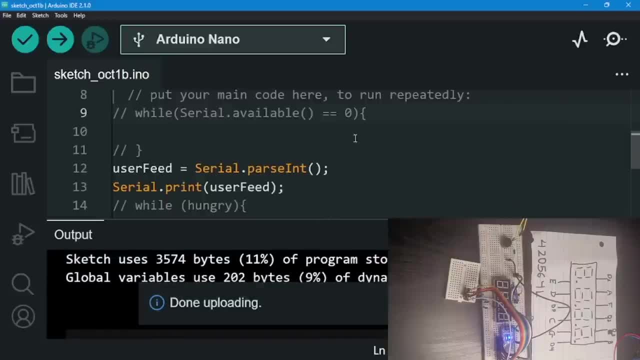 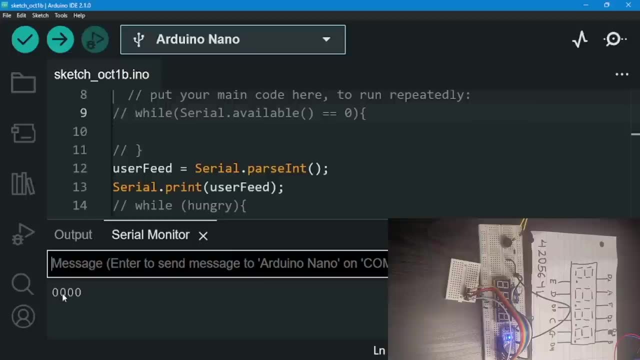 Okay, Let's see what happens. Okay. Okay, Let's see what happens right now. There we go And when we put on the serial monitor, let me just again, if she cannot see it right now. but it keeps on outputting 0, 0, 0, 0, 0,. can you see it? 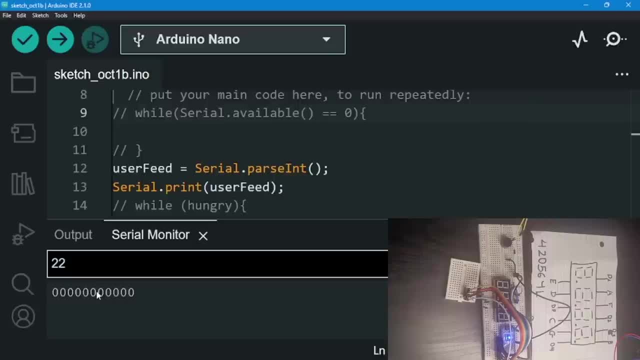 But let me just again give it a value right here. Let me just say 22.. Okay, It's going to output 22, and then it's going to go back to 0, 0, 0, 0.. What's going on? 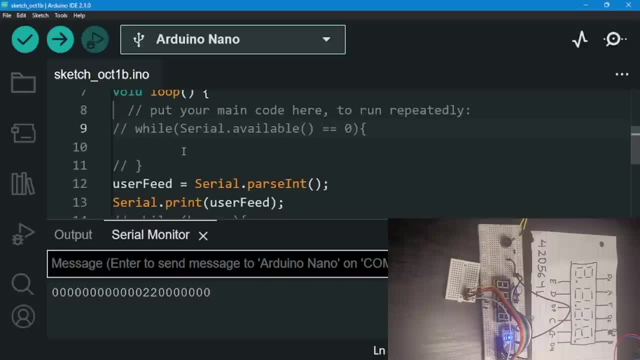 You might be wondering. obviously, the problem here is what. The problem here is what Arduino starts reading this code. And for now, what did we set in our, in our message bar? Okay, We did not set anything. When we don't set anything, what happens? 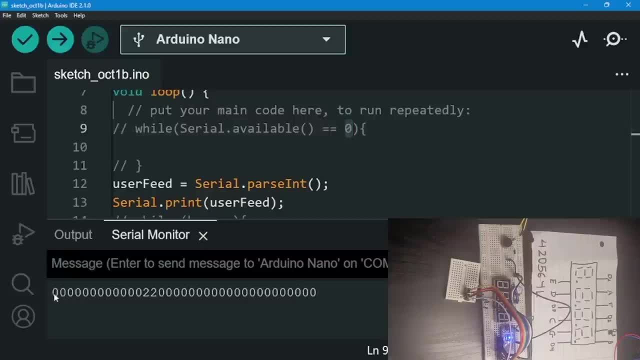 It's equal to what. It's equal to 0.. So, basically, what It's going to output, 0.. Can you see it? It's going to be outputting 0 and it's going to be printing it. You see that right. 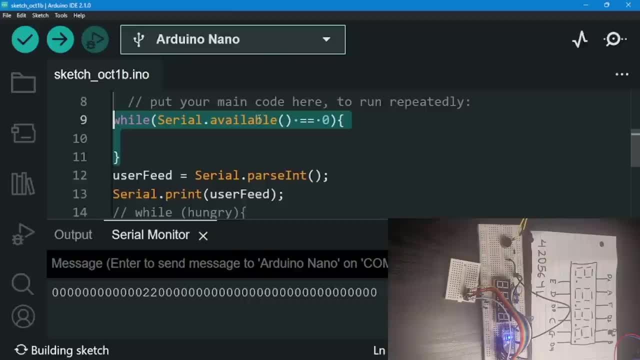 So what do? what does it prevent to This whileserialavailable again code prevents to it's going to wait for us, to what? For our message? before what, Setting up our variable. So it's important not only asking the question, for the question not to be repeated again. 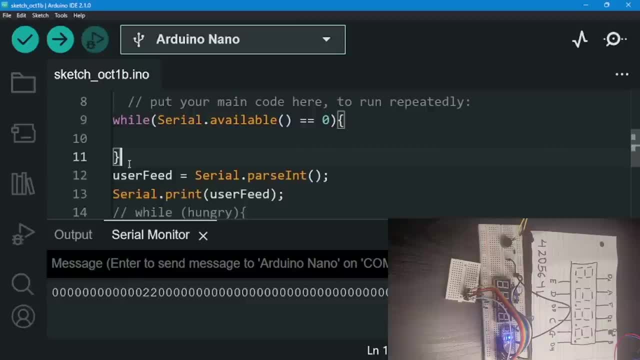 and again and again. but it's also important in what it's also important for us, to what To set up our variables. Okay, So it's just going to set it up to what it's going to be setting our variable before we give it a response. 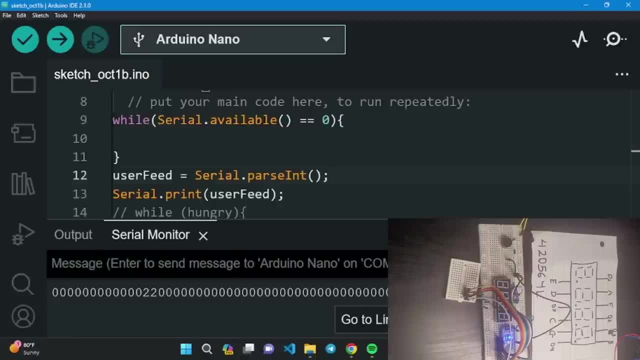 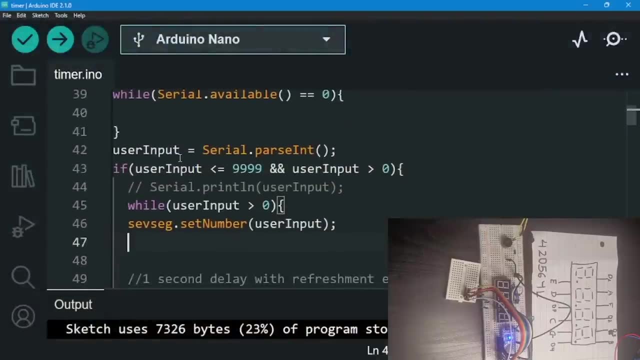 It's going to prevent that. Okay, So just keep that in mind. Okay, So let me just go over, uh, go over back to our main code right here and let's try to read the other part of it. So, right here. what I'm asking it is is user input, is what 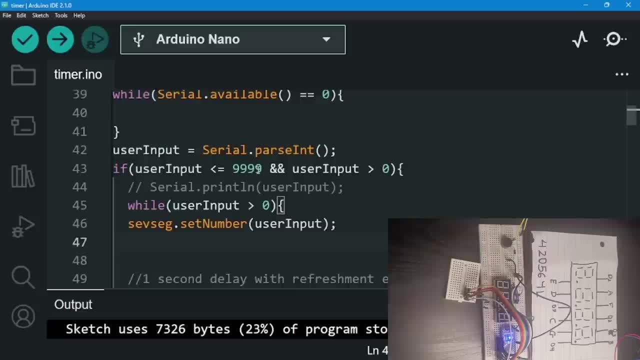 Less than or equal to 9,999, because we cannot display anything beyond what four digits, as I said again, and and this symbol right here. And then what? Okay, So the answer is what? user input must be greater than zero. 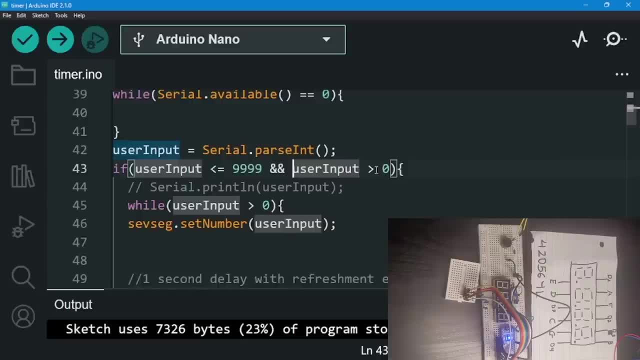 As you remember what it goes down, it goes. let's say, if you have 20 right here, we start our timer from 20.. It's going to go 20,, 19,, 18, it's going to go all the way to. well, let's say it goes. 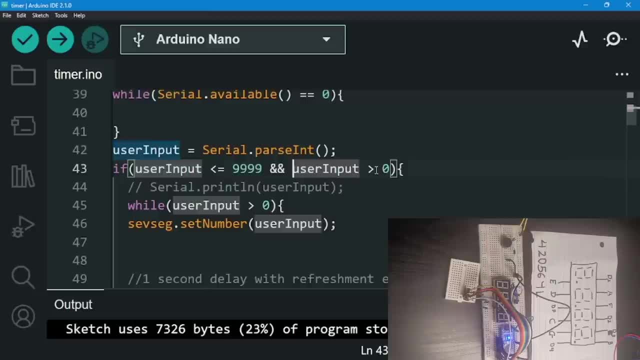 to 5,, 4, 3, 2,, 1, 0,. it's going to keep on decreasing. So negative one, negative two. I don't want it to go to what I don't want it to go to. 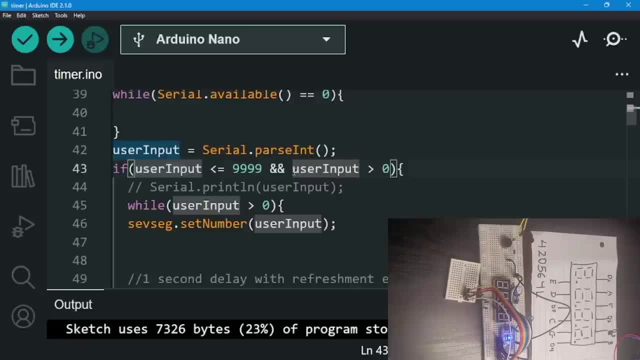 negative numbers and zero because obviously time obviously cannot be negative. Okay, So I don't want it to go to what Negative numbers? That's why I always want to check before running any code. I want to make sure that the user input is what has to be greater than zero, because we're 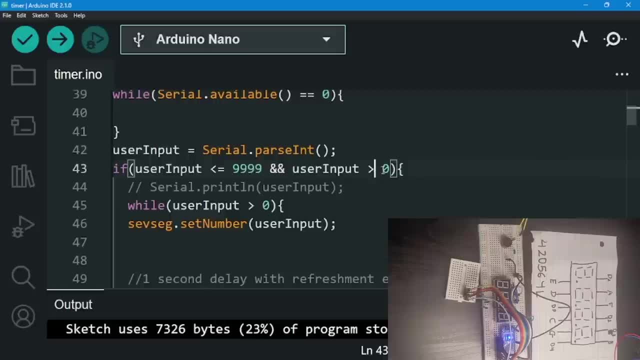 going to be what? we're going to be decreasing one as soon as we go. Anyways, one thing you always want to make sure is what's less than 9,999 and then what less than or equal to 9,999 and then greater than zero. 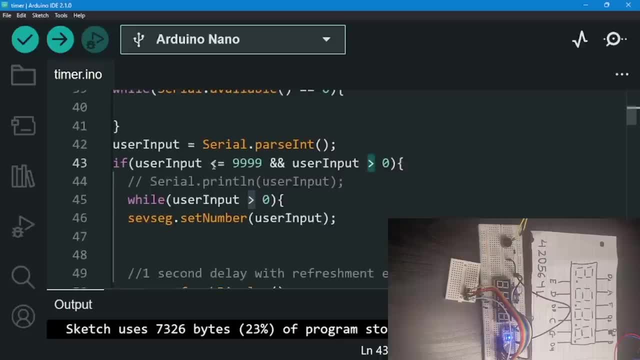 Okay, Then okay, These again, this symbol right here. let me start from the symbol right here. I think you guys know, obviously, the F statement. the symbol right here basically means less than equals to. If you just go over here, and let me just go over here right now and let's go to less than. 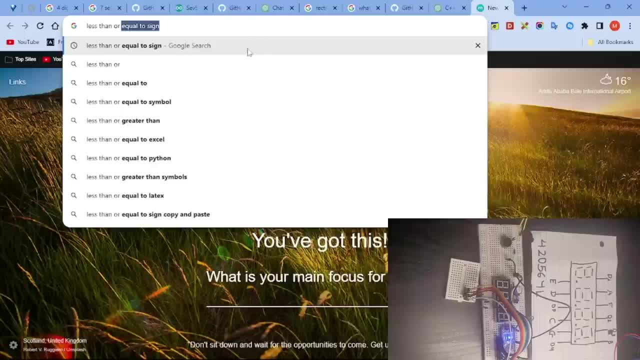 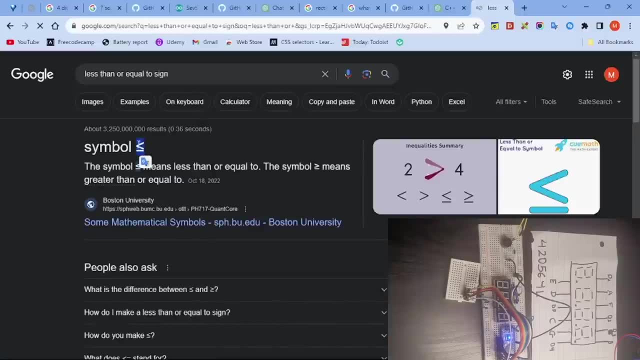 or less than or equal to the sign. If you look at the sign of it. I think most of you are familiar with this in math. We use this sign, this symbol right here, but we don't have the symbol in our keyboard. 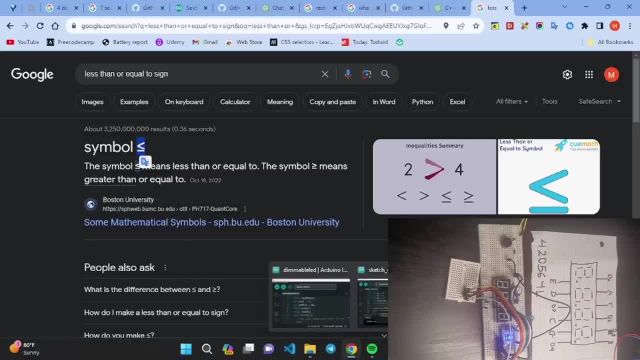 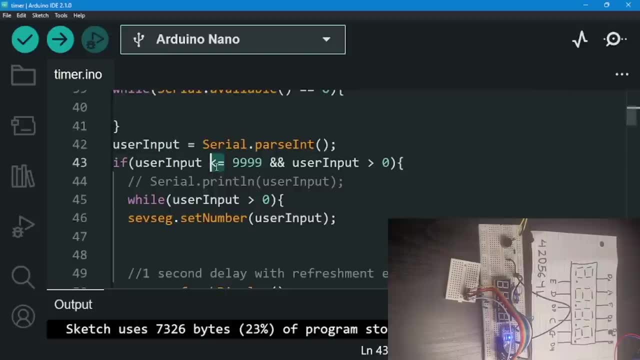 Okay, So I'm going to recording. We write it down, is okay. How do we write it down? We write it down as what we put our again, our first, again less than or equal to whatever it is less than or better than we put it first. 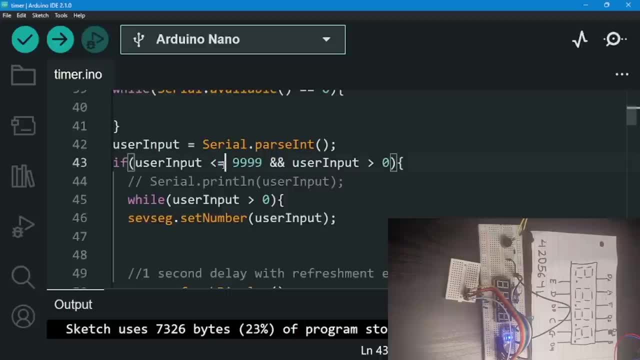 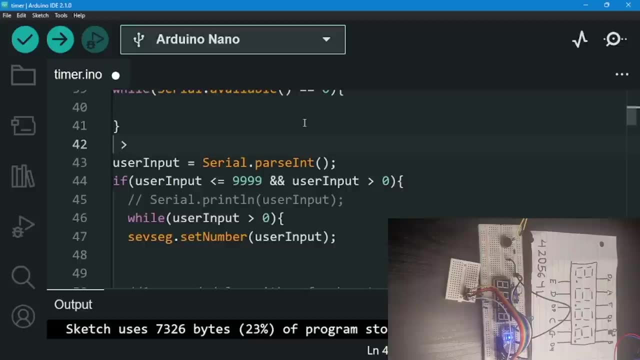 And then we put the equal sign. Okay, You put the equal sign at the end. Okay, So for something like greater than, let me just try to write down greater than. if you want to write down greater than or equal to, we just put the greater sign right here and 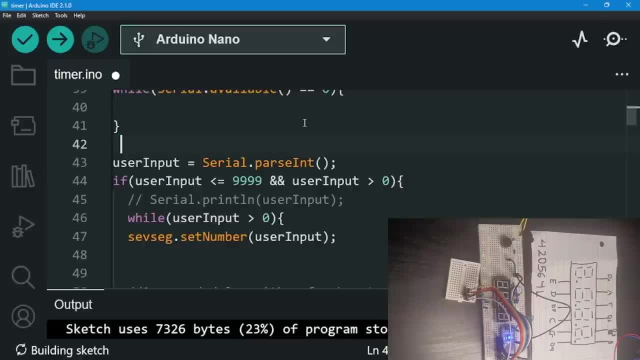 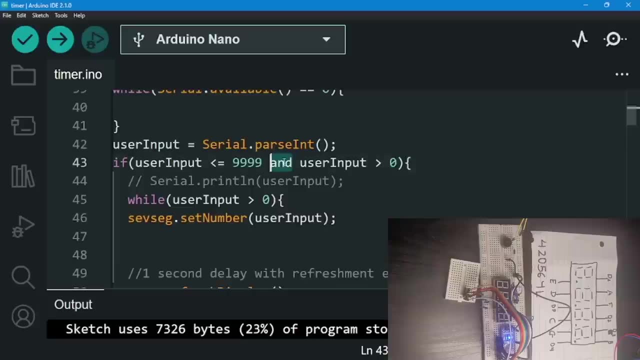 then we put the equal sign at the very end. Okay, Just want you guys to keep that in mind. Okay, And what does this mean? This basically means like the keyword and okay. It's basically means end. Okay, So right here, what does this mean is okay. 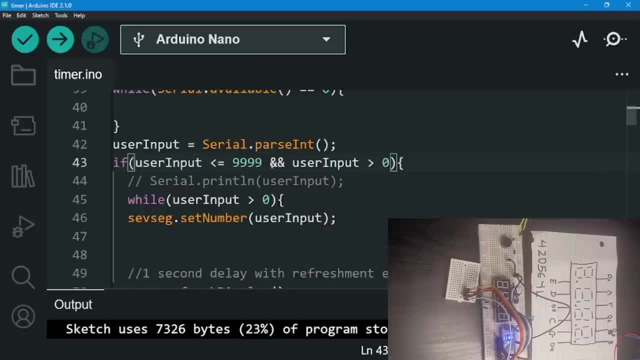 If the user input is less than equal to 999.. Okay, End. user input is greater than zero. It's gonna what? it's gonna run this code Basically if one of them is false. what happens if one of them is false? 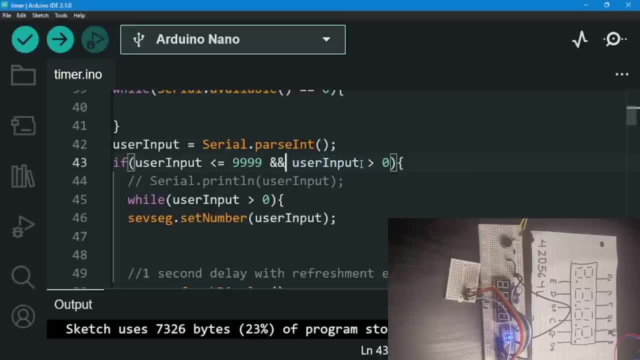 You know, let's say the user input is less. Let's say it's less than what is less than zero, Right here. Okay, Let's say it's even zero or negative number, And this is going to be true. User input is gonna be what less than negative? 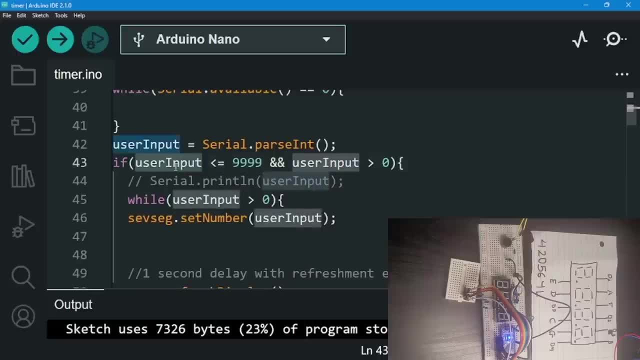 It's gonna be less than or equal to 9,000.. And then, because it's going to be a negative number, Okay, This is going to be true. But in this case, what happens? in this case, it's gonna be what it's going to be false. 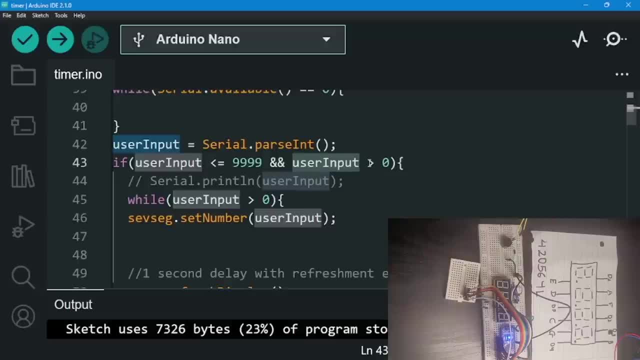 It's not greater than zero And negative numbers. now what greater than zero? So it's going to check what Both of them are true. So if only both of them are true, it's going to happen what. It's going to what? 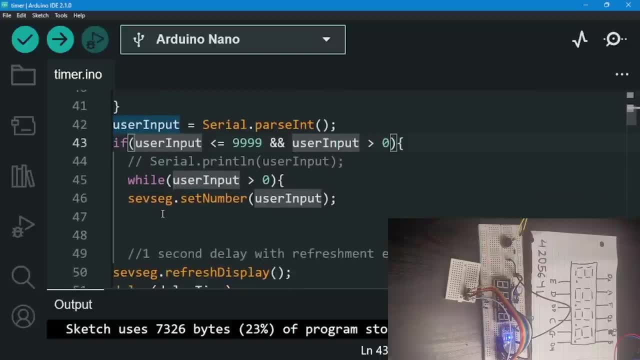 It's going to be running this condition. It's going to be running this code. okay, This condition is going to be true. if only both of them are true And we're using end. okay, That's how we express the logical term end. 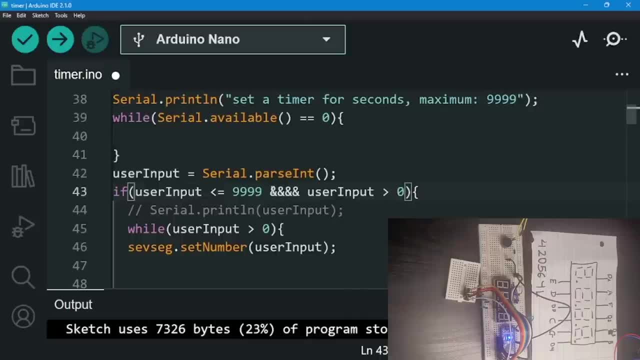 We just say: we put double what, We put the double end signs right here, and that's it okay. I just want you to keep that in mind When it comes to, or obviously, or when it comes to or. let me just actually go back here. 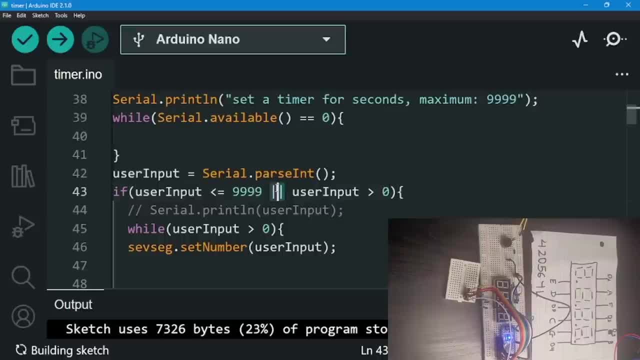 When it comes to, or we use this sign: okay, We use this sign that's found again above your enter key and you just use shift and then you just again touch it. Okay, so what does this do? 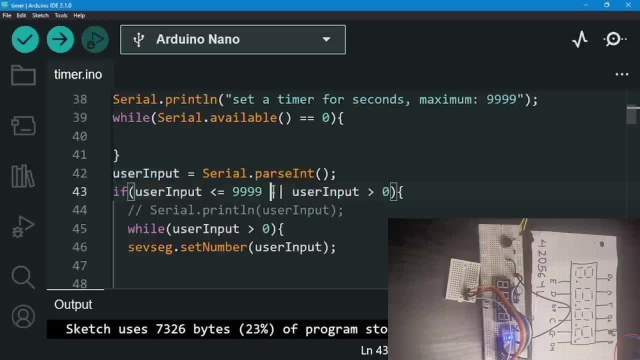 This basically means: or okay, And when it comes to, or one of the conditions are true. If one of the conditions are true, it's going to be true. So it's basically asking if user input is less than or equal to 9,099.9,. either this is true or this is true. 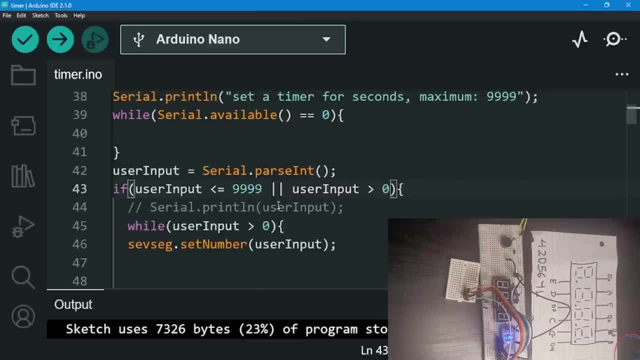 If one of them is true, it's going to run the code. This condition is going to be true. This statement is going to be what. This statement is going to be true. okay, I want you to keep in mind that this statement is going to be what. 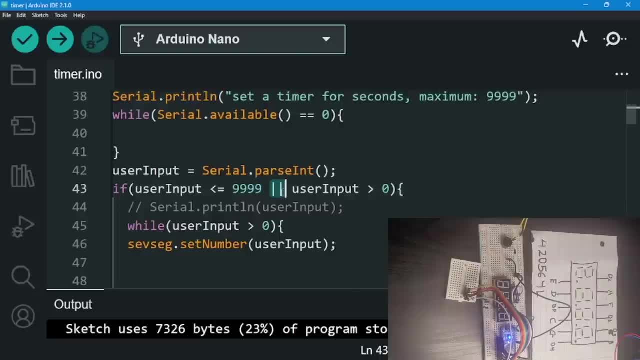 It's going to be true. So it's going to want what It's going to, only want one true value. okay, When it comes to the end, everything must be true. Everything must be true for the whole condition to be true. okay. 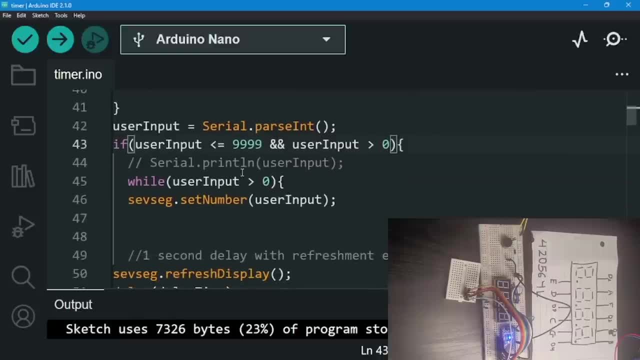 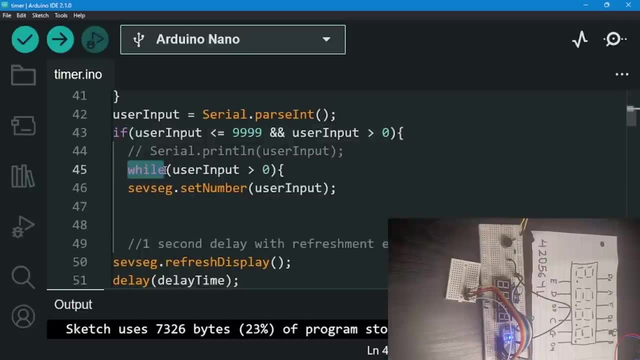 All right, just keep that in mind. Okay, now let me just go right here and again right here. we're going to be running the while loop. okay, So it's going to be going until this loop. until what? 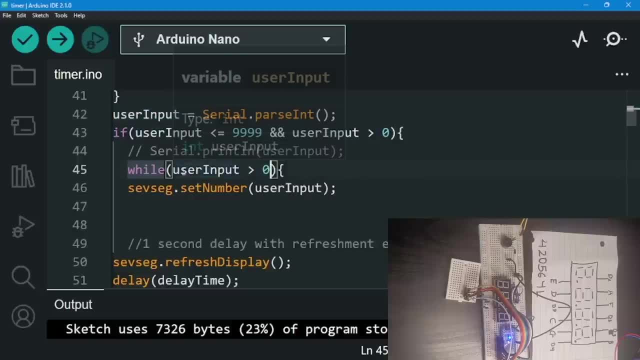 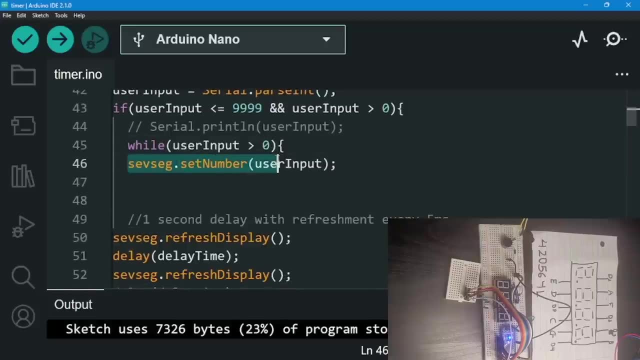 Until this condition turns out to be false. So we're going to be checking again. if this is greater than zero, okay, Just checks for zero. and then what happens? It's going to set a number. Basically, what it's doing is what? 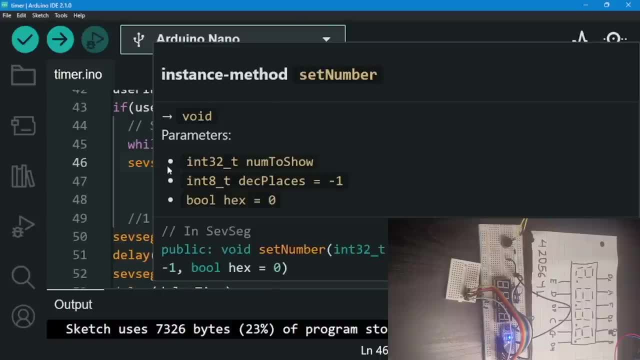 We're telling what We're telling CephSeg. hey, I want you to what? I want you to what? To display this number. okay, Set numbers. basically, I want you to display this number Basically. what is this? 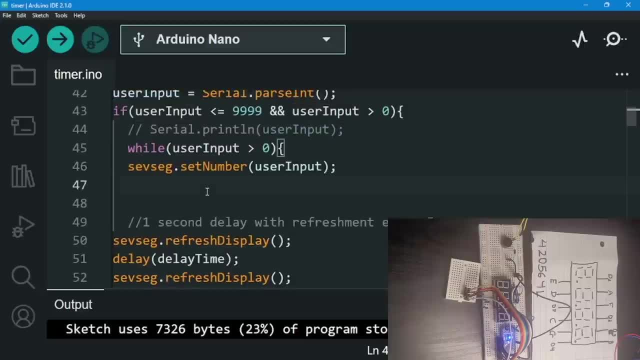 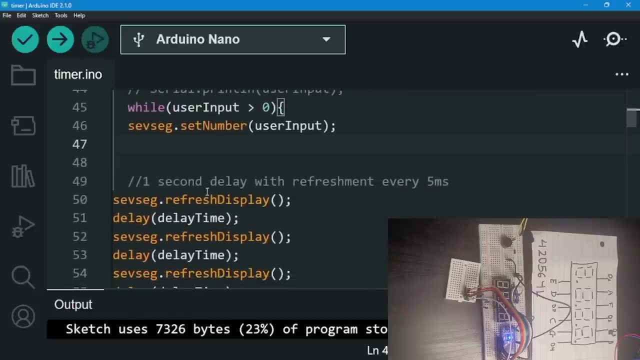 The user input Basically what the user just inputted. Okay, but once you're done doing that, what I want you to do is I want you to display it. okay, Okay, Okay, So let me just. there's a bit of a code that is repeated over and over again. 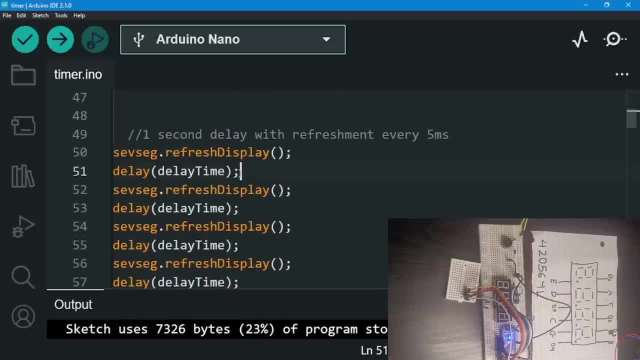 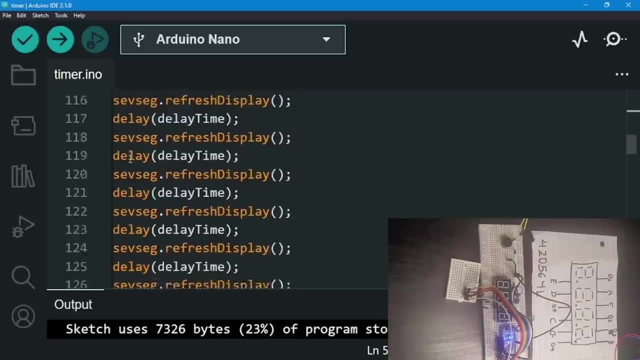 This code is repeated over like 200 times. okay, This code, like this specific code right here, this two lines, they're repeated again over 200 times. So you might be wondering why did we write this over 200 times? 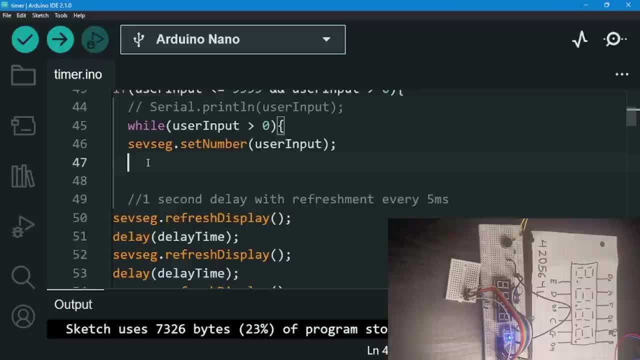 So let me just explain this to you. So, right here, what people would have suggested was: okay, I want you to do a CephSeg. I want you to what? I want you to refresh the display. So let me just explain what the refreshing display speed. 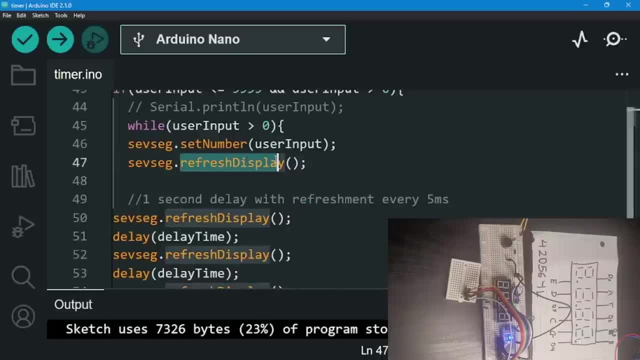 So refreshing display basically means when you're scanning again, you're again. if you remember, when we're using a four-digit again segment display what happens? We only turn on what, One digit at a time, So it's going to what? 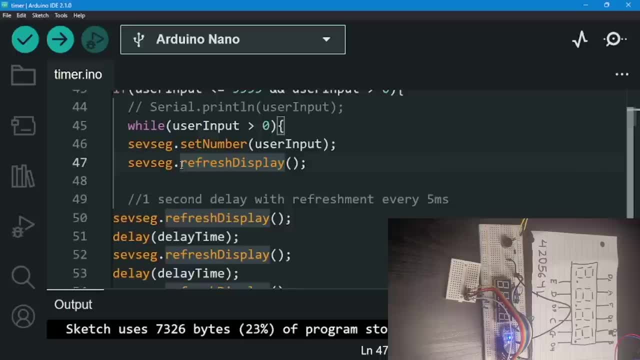 It's going to keep on scanning Basically what. It's going to keep on running the same thing again, again and again and again, very, very fast that we don't see it in our what, We don't see it by our naked eyes. okay, 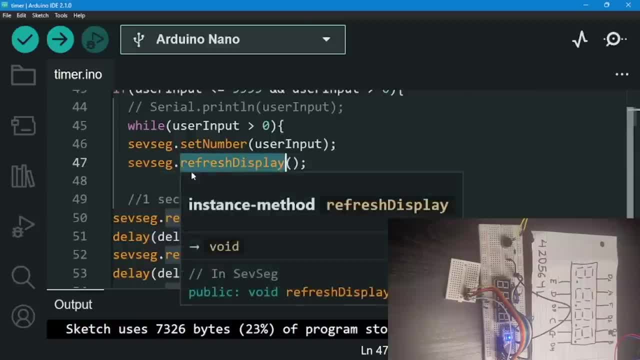 Basically, that's what's going on. So we're telling what We're telling. CephSeg, I want you to physically what. I want you to physically refresh the display. okay, I want you to do what. I want you to do exactly what. 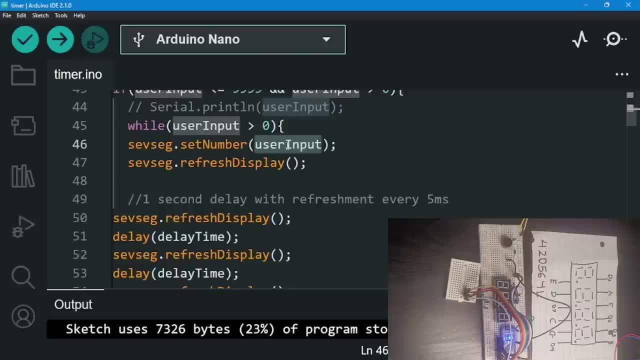 Refresh the display again and again. Let's say, for example, we put a number, for example, this time it's 20.. How do we display 20?? On the third digit, what do we do? On the third digit, we put a? what? 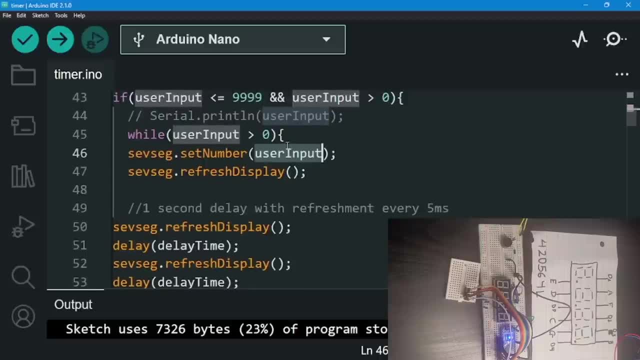 We put a two And then on the four-digit we put a what. On the four-digit again on the display, we put a what, We put a zero, okay. So I want it to what? I want it to basically refresh the display. 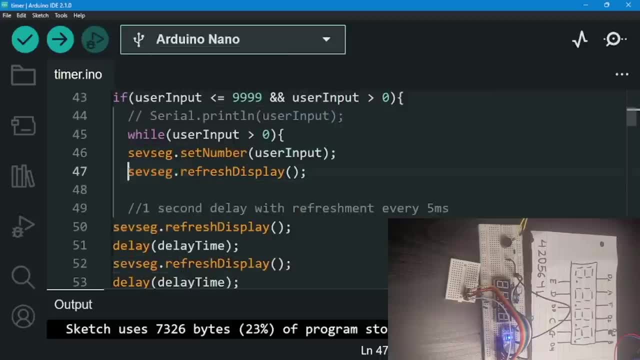 I want it to go from two zero. I want it to go two zero, two zero again, because we can again, as i said, again, we can only turn on one what? one digit at a time. so it's going to do it very fast. so step seg is going to automatically what it's going to again when. 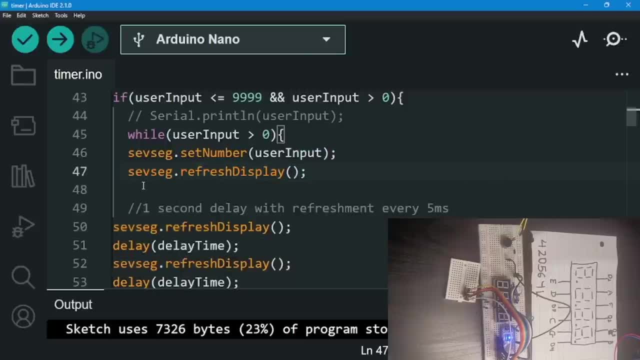 you tell it again, it's going to what? it's going to refresh it again and again. okay. so most people would have suggested- just me, let's forget about the code that's beneath here. okay, so beneath the comment, right here. so what most people would have suggested was refresh the display and then okay. 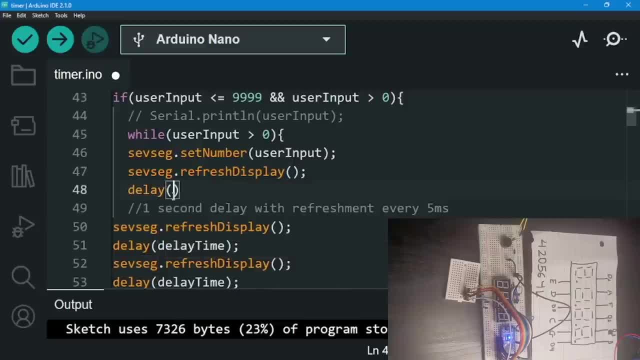 you know what we have to set a delay for what? for one second. why is that so? basically represents what after one second. we just wanted to what we're basically what? representing one second of delay right here, one second, and then we're gonna do what? we're gonna decrease it, okay. 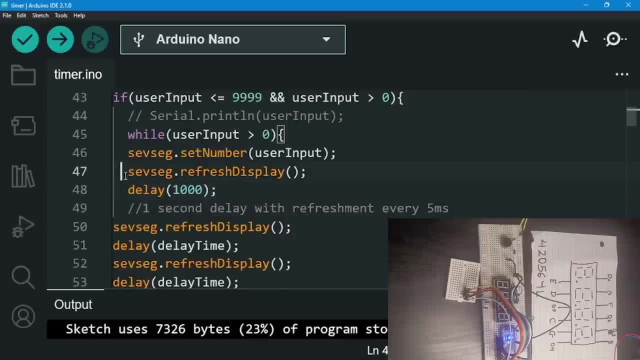 that's what's basically what, uh, most people would suggest right here. we're gonna be telling what: refresh the display and then delay it for a second so that it counts what it counts a second. okay, it counts a second on the timer, and then what it can. again, we can keep on what we can keep. 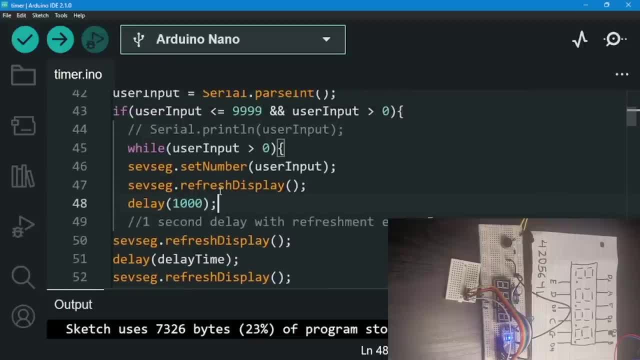 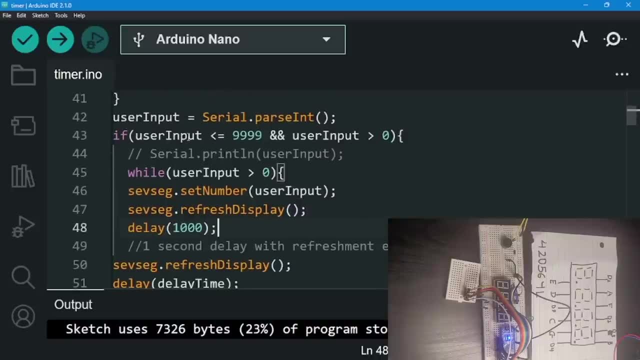 on decreasing the user input value. okay, the problem arises here. so, okay, let me just, let me just think that arduino is again reading this code, so it's going to go right here and let's see: the user input is what less than or equal to 999? yes, it is, let's say. i just 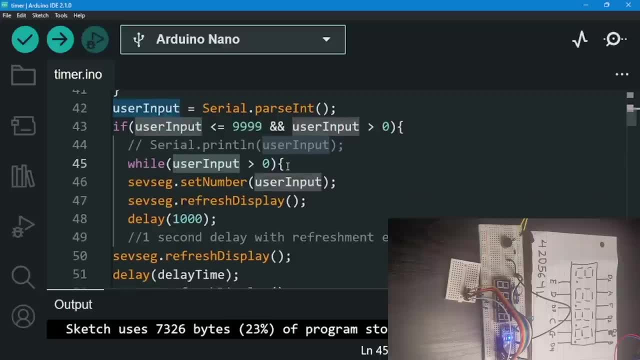 put 20 right here. okay, and it's 20 greater than zero. yes, it is. so. it's going to read this code and then it's what it's going to be set the number to. what it's going to be setting the number to 20. 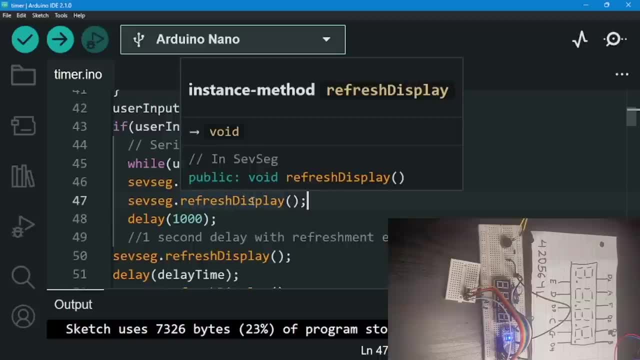 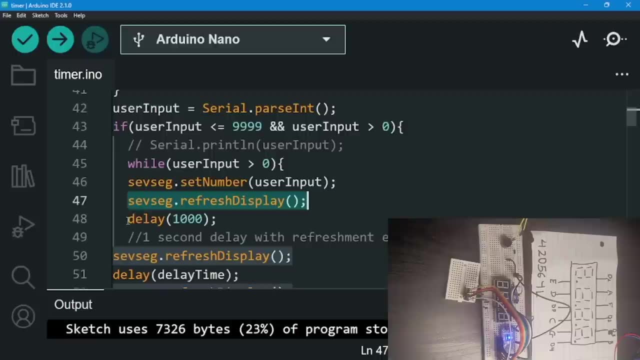 and then what? it's going to be refreshing the display, and the problem arises here. it's going to read this in an instance. it's going to read this in number, in milliseconds. okay, it's going to refresh the display in milliseconds, and then it's going to be delaying. okay, physically it's. 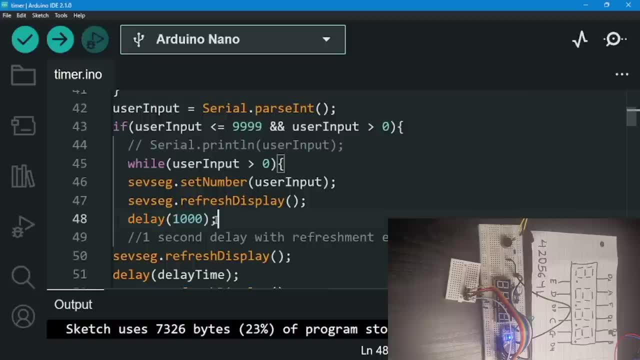 going to be delaying for what for one second? so it's going to turn off the display and delay for what for a second. so let's just say this again: takes arduino five milliseconds to read. let's just say it takes it definitely less than that, but let me just say it takes it only five milliseconds. 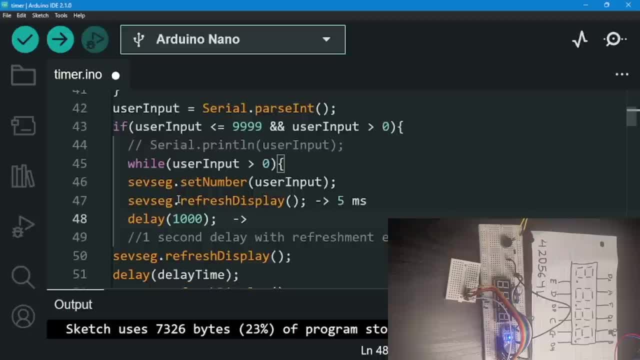 to read this. okay, how about this? it's going to be spending. okay, it's going to be what? it's going to be turned on for five milliseconds and then what happens is what? for 955 milliseconds, it's just going to be off. okay, it's going to be what? it's going to be delayed. okay, it's going to just going. 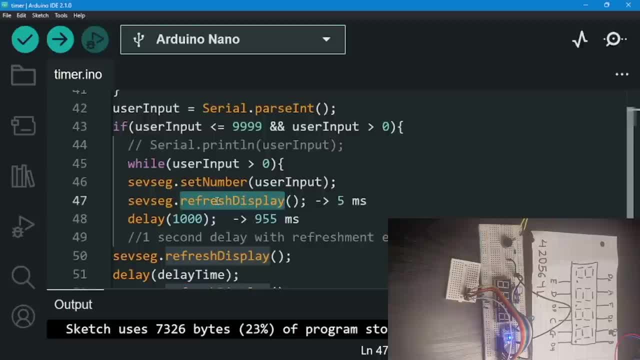 to be delayed. it's not going to be on. okay, we're not going to be refreshing the display and then it's going to be just delayed. it's not going to be reading any quote, for what? for one second. that's what's going to be going on, okay. so what is the right way of doing things? okay, what's the? 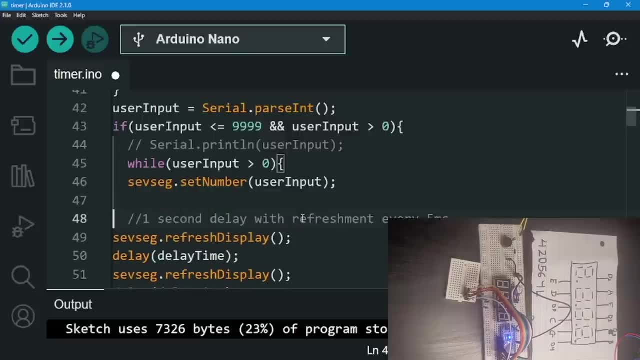 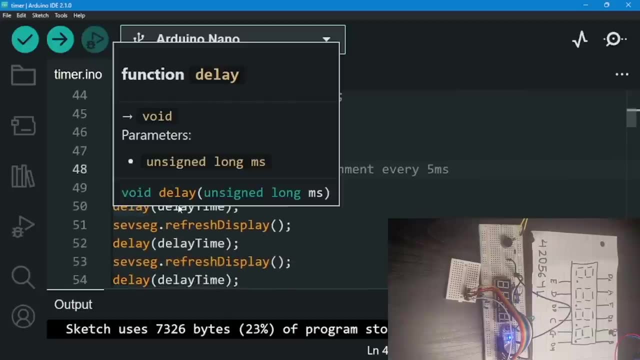 right way of doing things, then the right way of doing things. let me just remove this code again. the right way of doing things is okay, we're going to put our self sake, we're going to be refreshing it and then we're going to be delaying it for five milliseconds because we cannot notice five. 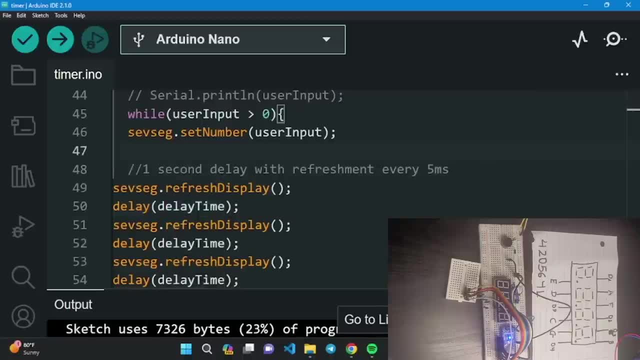 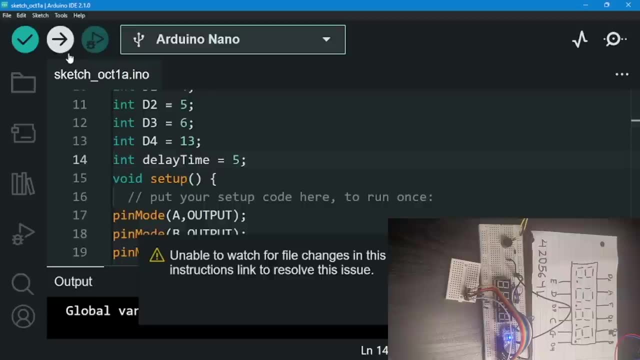 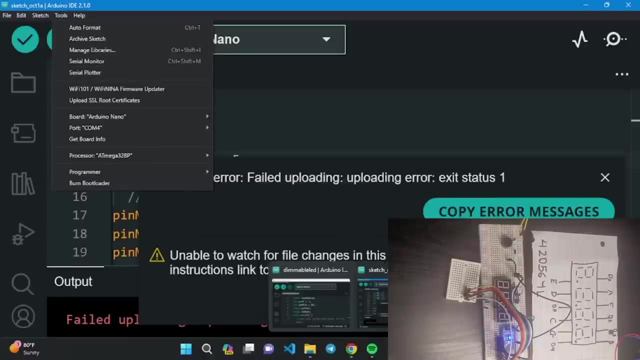 milliseconds when i put everything as i said again, let me just put this right here. where is it there? the delay time here to 5 and we again uploaded the code. Let me just upload it. Okay, there we go. It failed to upload. Okay, I see. I see why it failed to upload. Let me turn off. 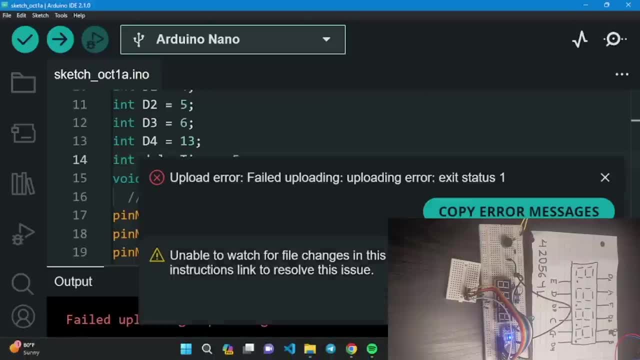 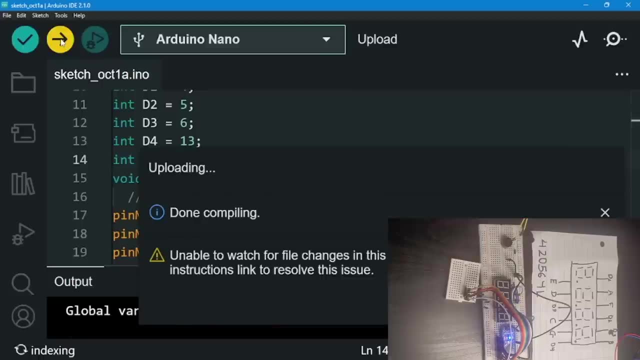 my serial monitor right here. There we go. Let me just upload this. Forget about the errors right now. Okay, I should be done compiling and uploading. If I just upload this right now, can you see it? It's going to go so fast that we cannot see what. We cannot see a change. 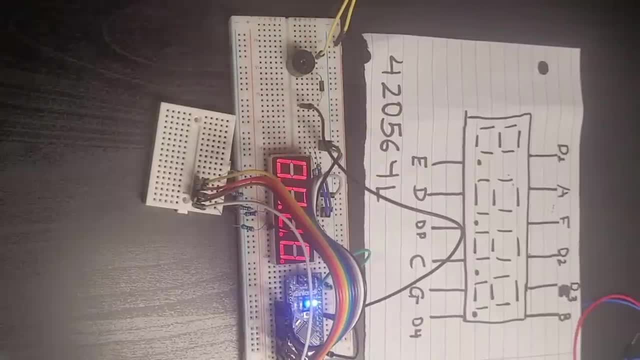 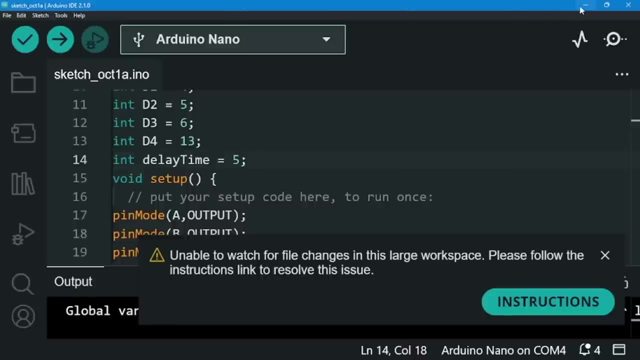 from one digit to another digit, change from one digit to another digit and another digit. Again, we cannot see it, because it's going to what Very fast- 5 milliseconds is just so fast for our eyes. Okay, so what I did was let me go back to my again normal code. 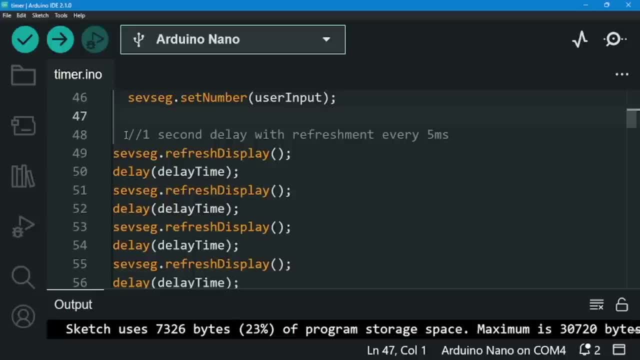 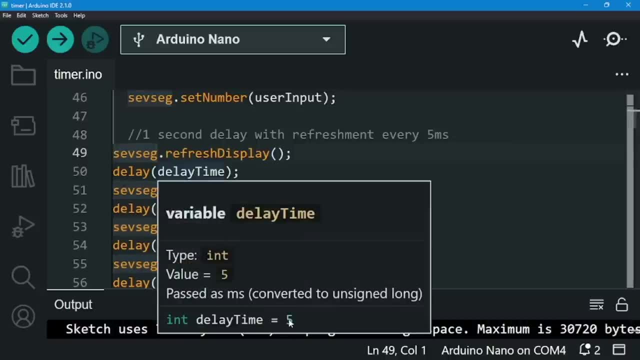 right here. Okay, what I'm going to do for my normal code right here. And then what do I do is I keep on refreshing the display and I keep on delaying it by 5 milliseconds. Okay, I keep on delaying it. by what? By 5 milliseconds. There we go. So I keep on refreshing the display. 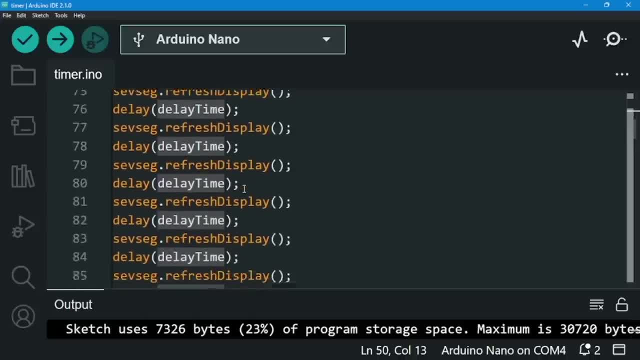 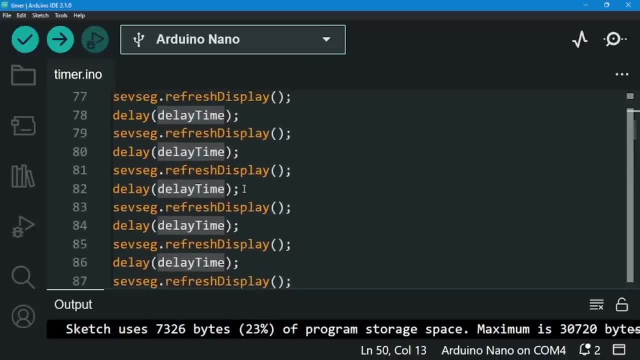 and doing it how many times? 200 times. Okay. this code is again reading over and over again. So it's reading like over 200 times. Okay, if you go all the way up to, I think, line 400 or something, you can see the end of it, But anyways it. 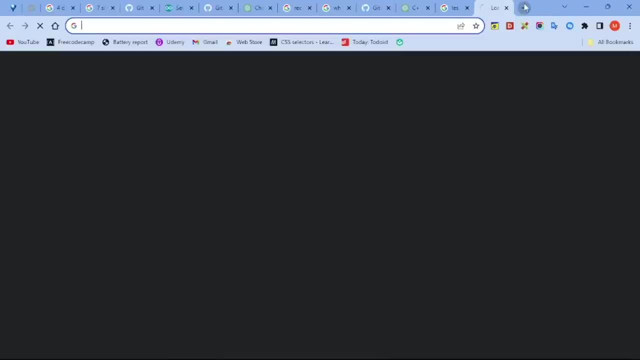 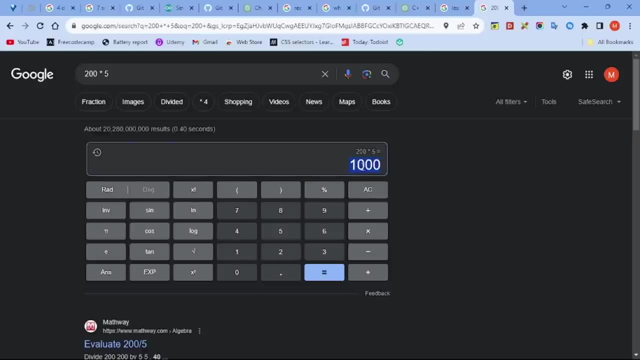 was written 200 times. So obviously the simple question is: what's 200 times 5?? 200 times 5 is what? 200 times 5 is 1,000 milliseconds. Basically, what? Basically a second Okay. 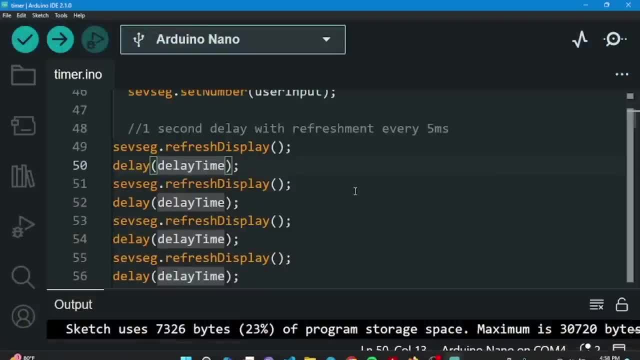 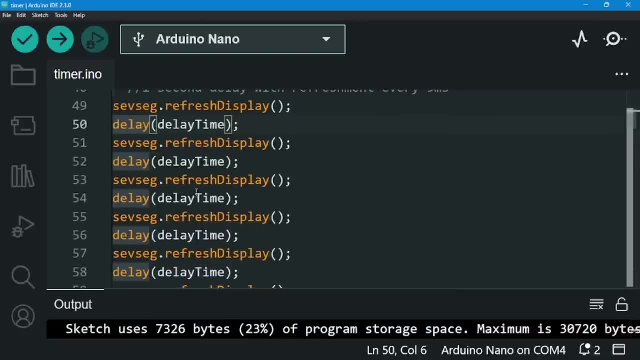 that's one thing I want you guys to keep in mind. So, right here, I just keep on refreshing the display and then do what? Do? a delay of 5 seconds Refreshing the display. I keep on doing this over again 200 times. So how do we do this? Obviously, again, you write down. 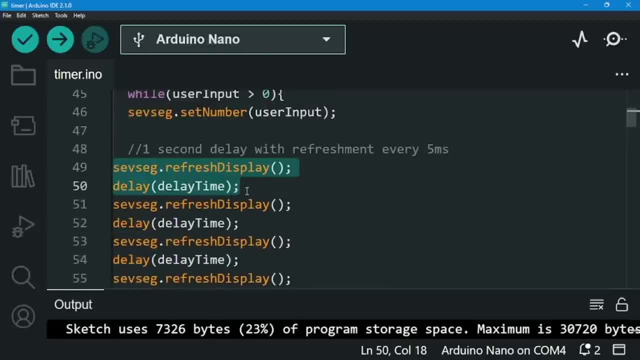 what I did was what I obviously wrote down this code right here And then I started to copy paste it until again, to the point of where it reaches 200.. Again, you have to get pasted 200 times. I think you guys know how to paste this 200 times really easily, Obviously. 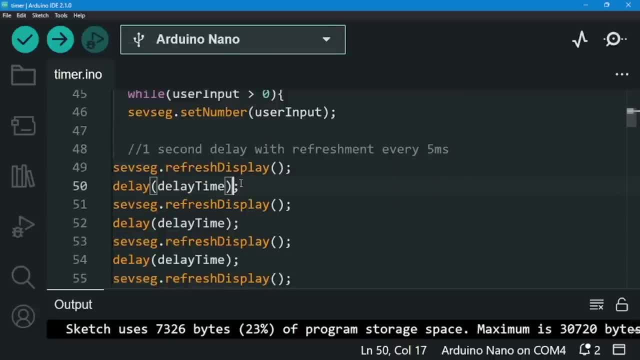 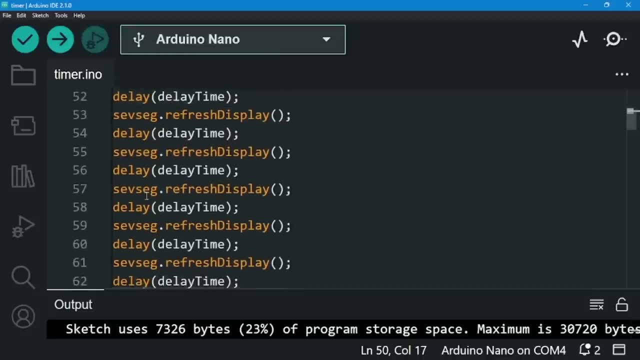 what you do is what: You write it down and then you paste it until it's 10.. And then you copy the whole 10.. And then you paste it until it's 10.. And then you copy the whole 10.. You paste it how many times? 20 times. So basically, you just count up to 20.. And then 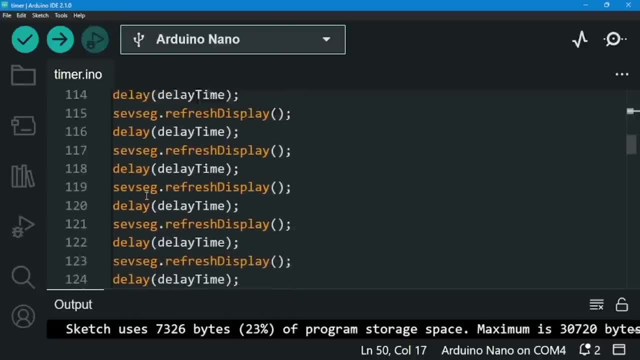 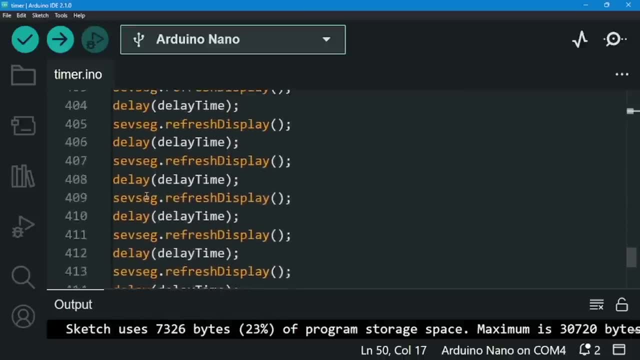 it's what? It's 200.. Okay, so you obviously don't have to paste it 200 times. Okay, I don't have to paste the same to these two lines 200 times. There's an easier way to do it. Okay, so right. 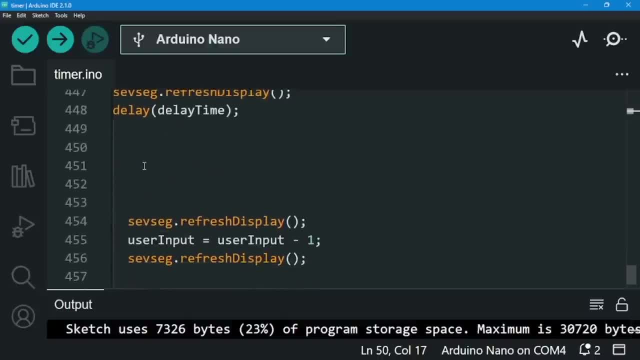 now let's go here. There we go. It ends here, And then, once I'm done, again again, displaying again my what I'm done, displaying the user input. for how much? For a second, for a total of one. 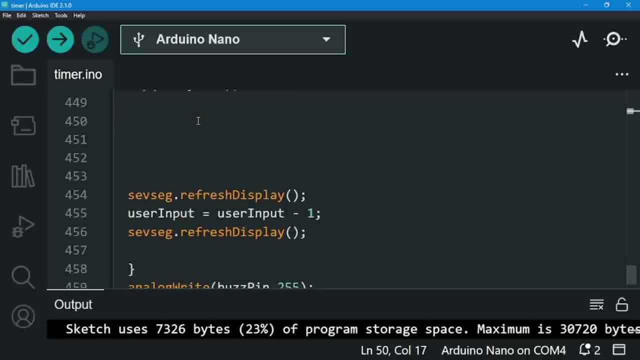 second. This adds up to a second. I told you guys, once I'm done doing that I want to do is what I want: a minus one from the current value. So right now, I said it was 20, right, So it's going to. 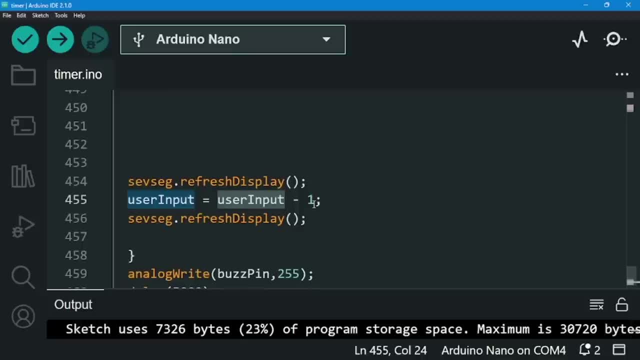 what Minus 20.. It's going to be 20 right here. 20 minus one is what It's going to be: 19.. And it's going to set it to what To the user input. It's going to set it to what To the user input. 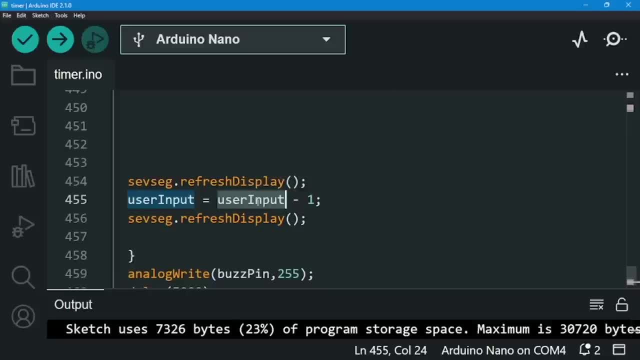 The new user input is going to be what? It's going to be the old user input right here, minus one. Okay, so it's going to be what? If it was 20 right here, it would have been what? The old, the new. 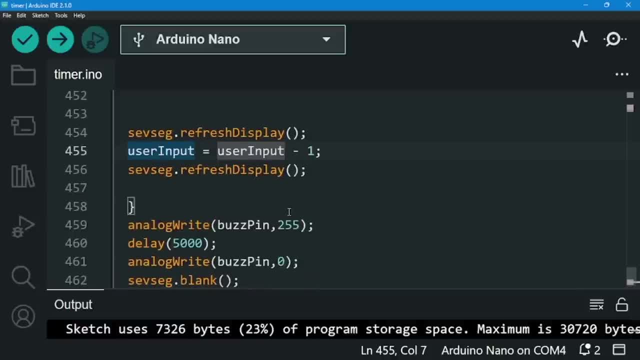 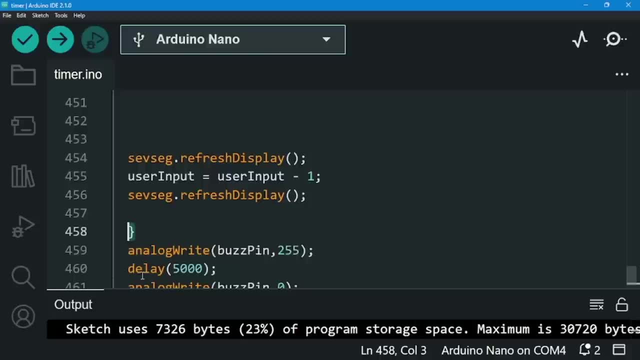 user input. So after we're done with that, it's going to what It's going to: refresh the display again. all right, And then what I wanted to do again is keep on running this while code. okay, We do not finish the while code right here. This is a code for another one, but it's going to keep. 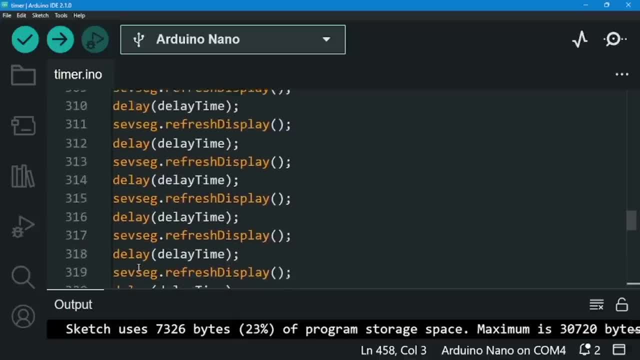 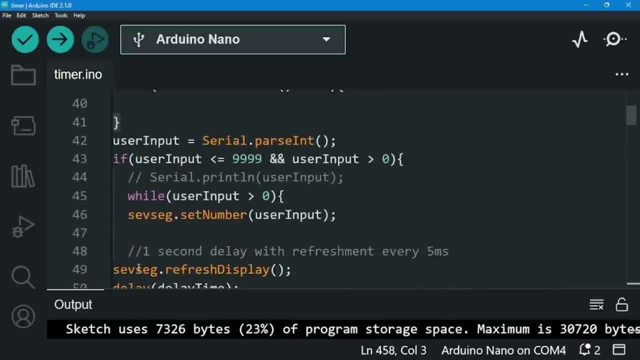 on running this while loop again. It's going to keep on running this loop over and over again until we reach what? Until we reach zero, Let's go all the way up. There we go. It's going to keep on writing this over and over and over. until what? Until we reach zero. As soon as we reach zero. 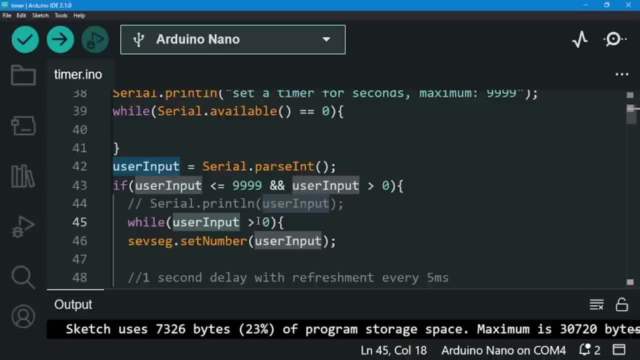 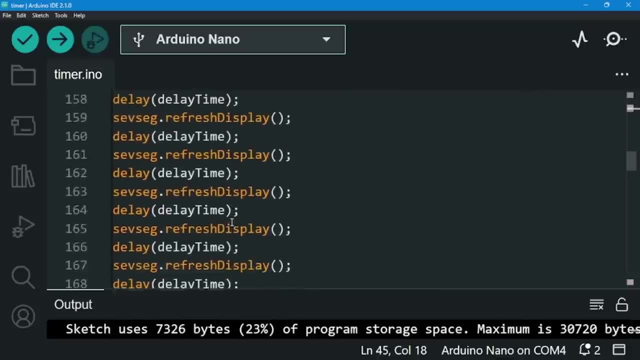 it's going to be. zero is greater than zero. Is that a true statement or a false statement? Is zero greater than zero? No, it's a false statement. And as soon as it hits zero, what happens is what? Again all of this code, all of this, that is, multiple lines, again. 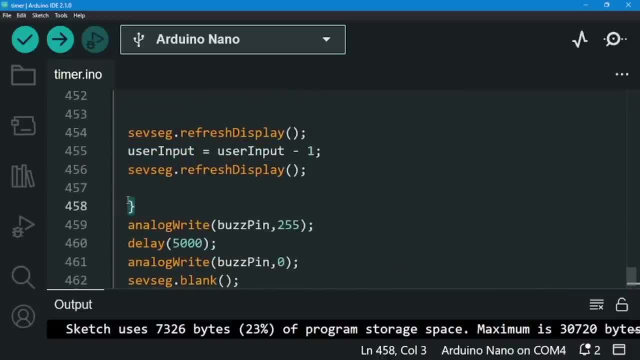 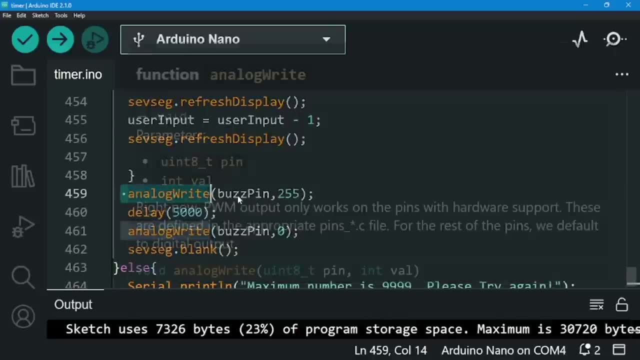 until the end of the curly bracket is going to be what. It's going to be skipped, And then, as soon as we reach zero, what happens is what? As soon as we reach zero, we're going to have what An analog right, Basically what We're going to turn on our what Bus pin for five seconds and 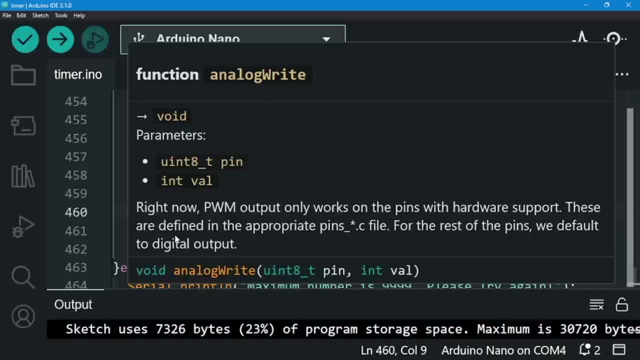 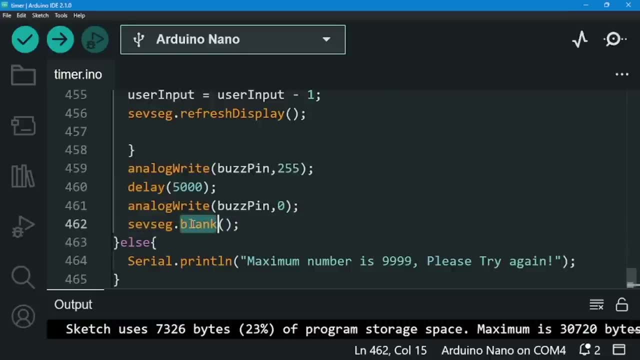 then we're going to turn it off, okay. So it's going to be ringing for five seconds and then we're going to turn it off. okay. Then afterwards, what happens here? Sebsecblank? what does it do, Sebsecblank? what it does is basically it turns off every what. It turns off the display, okay. 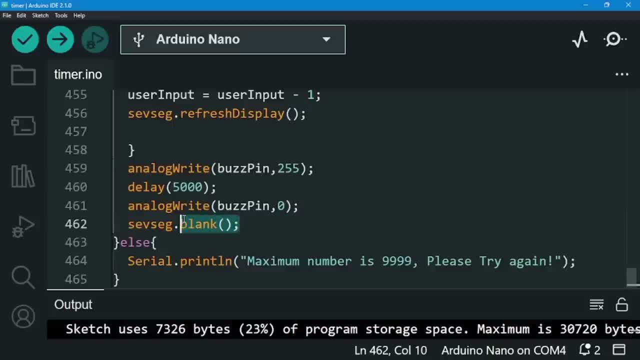 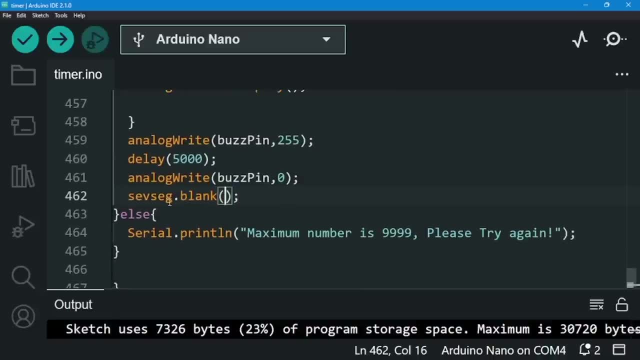 So, basically, if it was displaying anything and if you just put blank at the end, basically does what? It's just going to clear out the display, okay, It's going to be turning off everything from the display, okay, So right here, we're done with that and we're left with is only else. So, 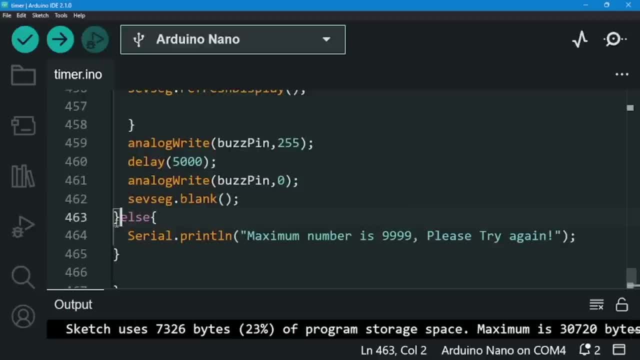 it's just the if-else statement right here. okay, If you want to see, by the way, the end of the curly brackets, right here, you have the rectangle right here. right, You have to find the other rectangle, the one that is what, The one that is highlighted by a rectangle right here. So this: 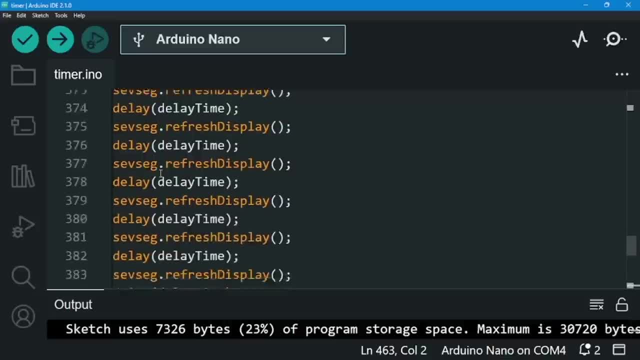 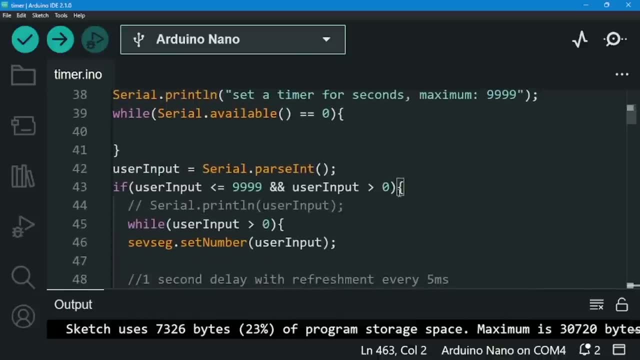 one is highlighted by a rectangle. Let me just find the other one that is highlighted by a rectangle right now. Let me just go all the way up and as soon as I do that, there we go. Can you see it? It's what It's mapped with a, what It's highlighted with a rectangle right here. So basically what? 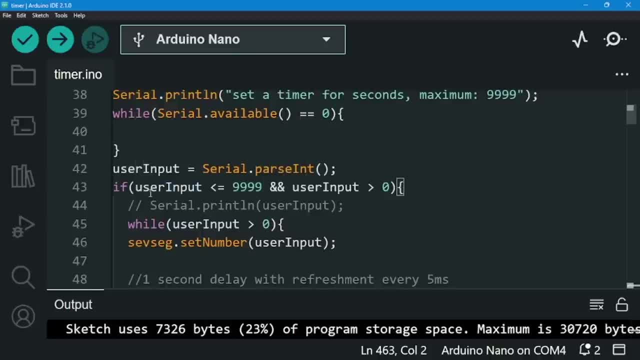 It's basically the curly bracket of what The if statement right here. So we're saying: if it's 9,999, and again, if it's greater than or equal to 9,999, and if it's what? If it's greater than zero, I want you to run this. 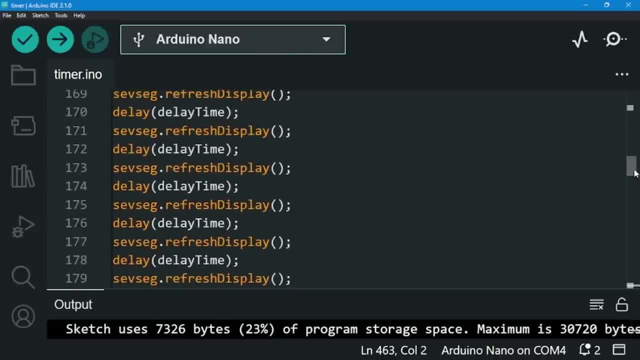 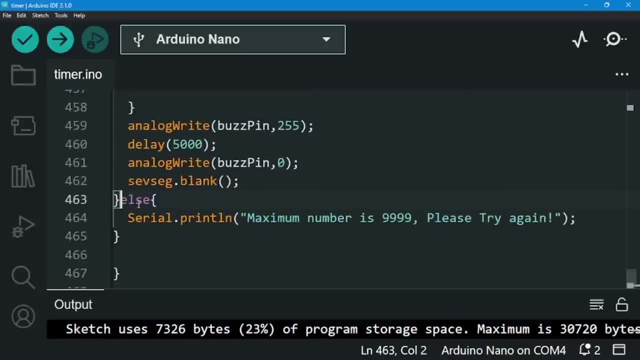 code. But if it's not, there's the else right here, The else. let me just go all the way down because it takes a long while. There we go. If it's not, you know, if it's not in this range. 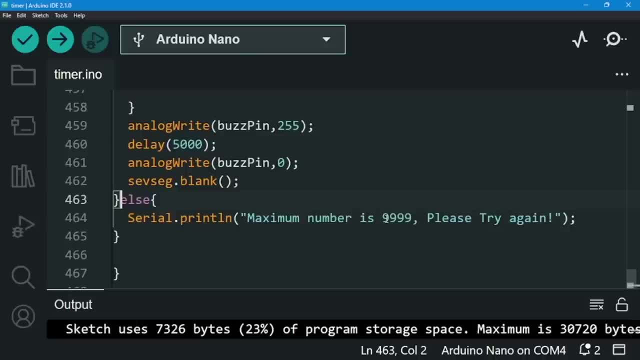 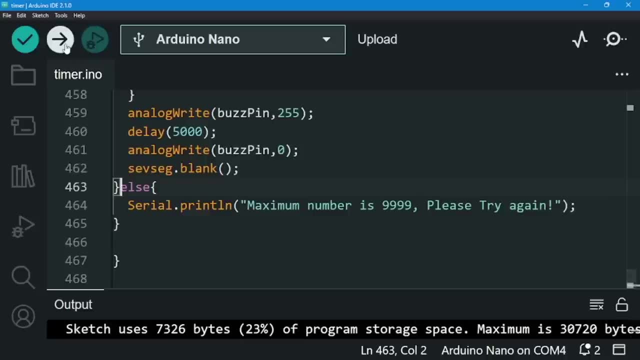 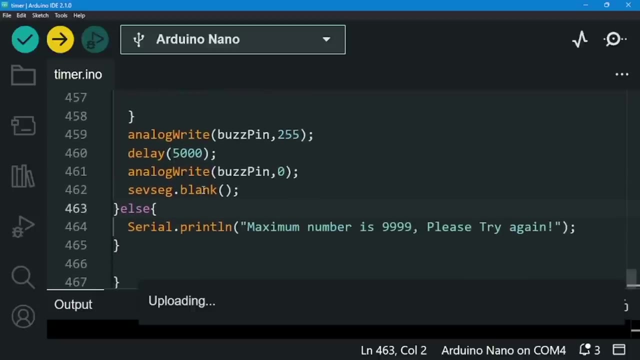 what am I going to say? I'm going to say: its maximum number is 9,999.. I'm going to tell the user: please try again. So let me just run this code right now. Let's just upload it, Okay. All we need to do is upload it right now, And now it should be working like magic, Okay. 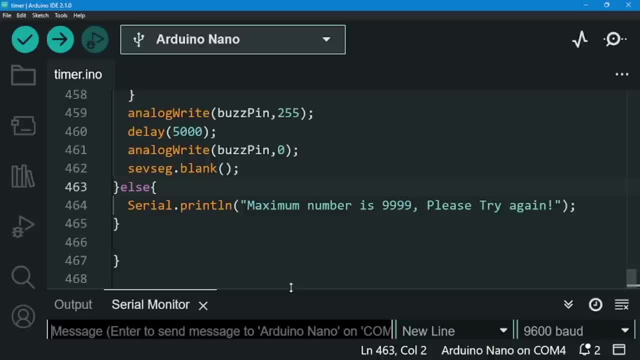 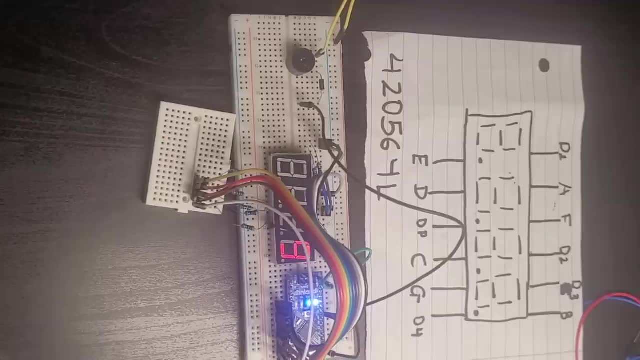 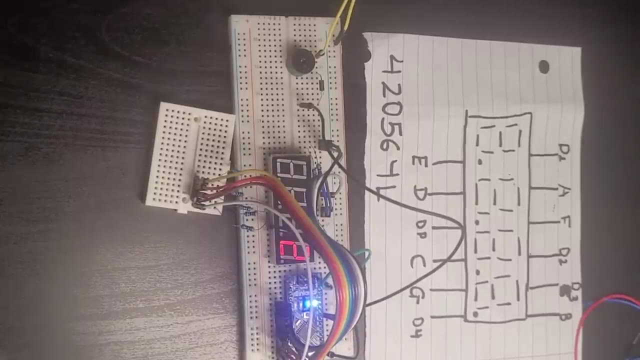 And it's done uploading, And now it should be working. There we go. Now. let me just say 10 seconds Should be counting to 10.. Actually, I can turn off the lights too. Yeah, that's nice. Goes to three, two, one. 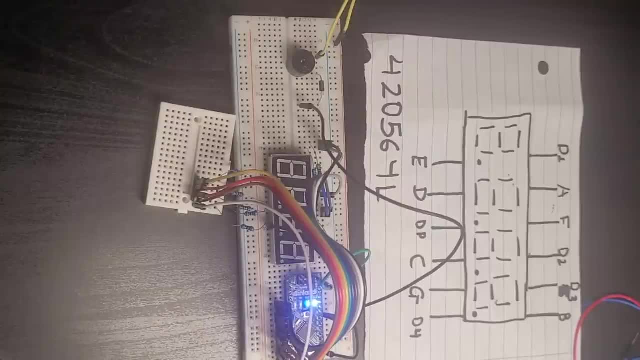 And there we go, The buzzer rings for what? For five seconds, And then what It basically turns off. So there you have it. This is a timer, again made from what? From four segments, LED displays using the what, The save seg again, library, Anyway. so this is one of the finer. 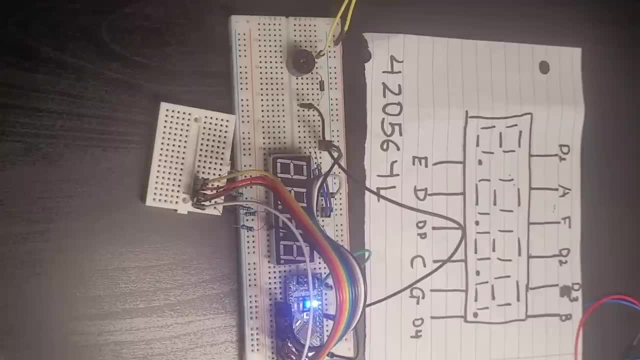 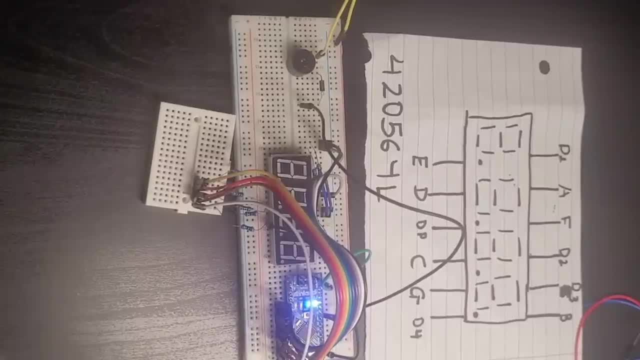 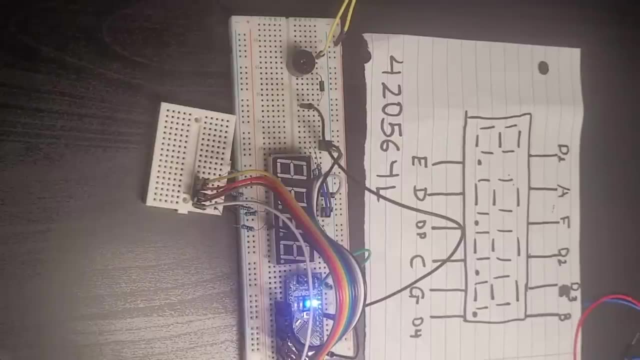 course, This is one of the hardest sections and actually one of the one of the most rewarding and one of the best- again, one of the best projects of this section of this, Sorry, Pсе course. So, anyways, I'll see you in the next section. 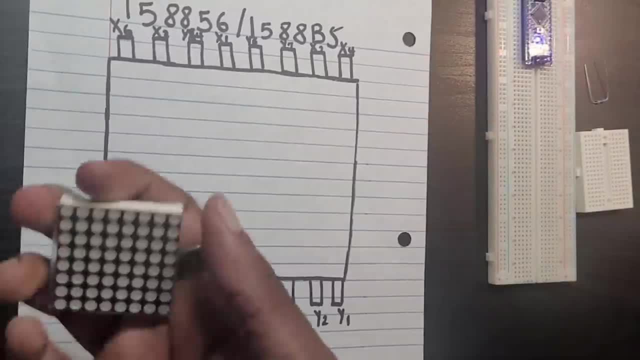 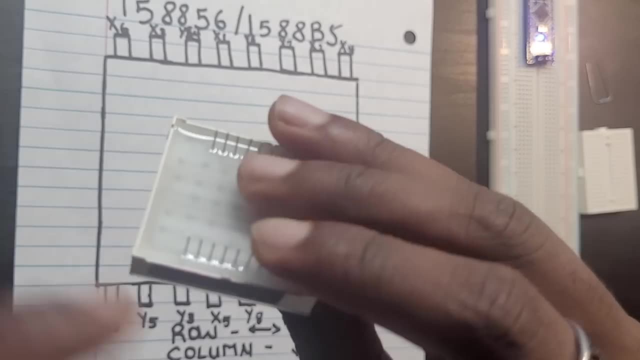 In this section we're going to be discussing about led matrices, So you're going to be looking for, I guess, these dot looking type of pins right here that have around eight pins here. okay, they have eight pins here and they have eight pins here. 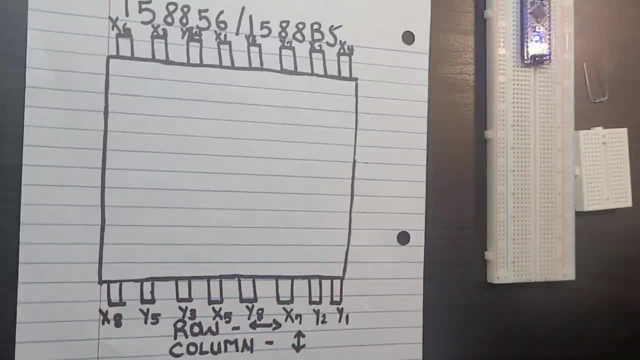 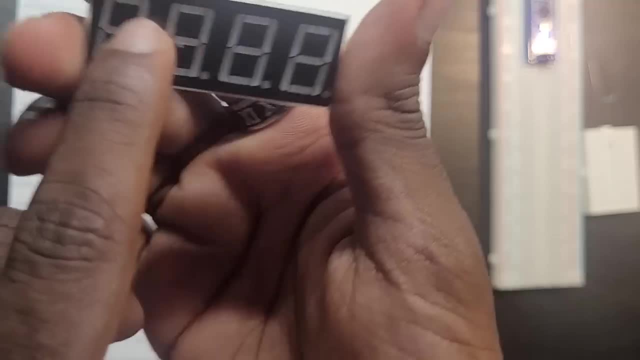 so we're going to be looking for something like that, okay, so one thing i want you guys to keep in mind is, while we're also working with the, with the four segment right here- so sorry- the four digit seven segment led display, one thing that obviously we had was the number right here, so it 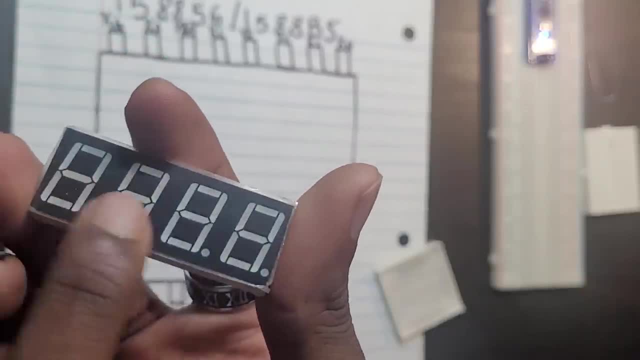 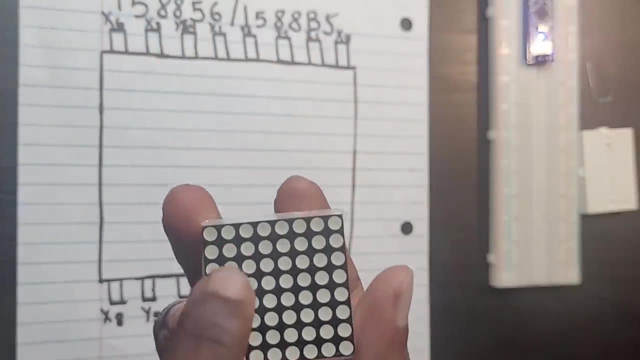 varied again. the positions of the pins varied again according to the number. one thing i want you guys to keep in mind is, again, there's going to be a specific number associated with your what with your led matrix right here, and then that number again is going to what it's going to be. 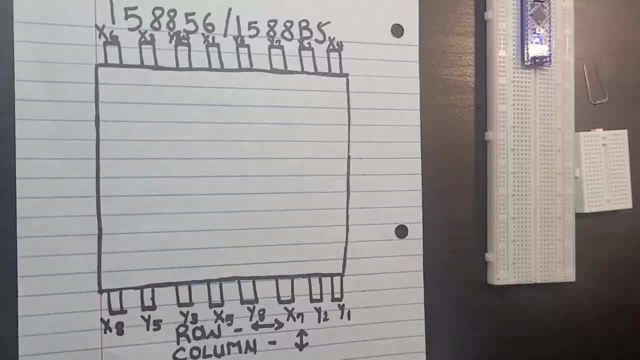 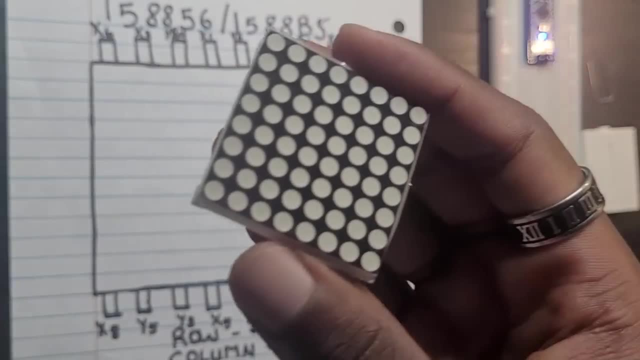 literally dictating which pin is which pin. so first on, let's just see what led metrics are even capable of. so if you've seen led metrics, it might look like something you've not seen before, something that is completely new. but if you again, let me just go over to my screen and i think most 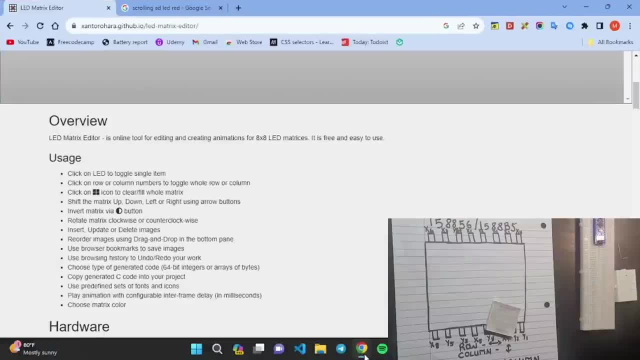 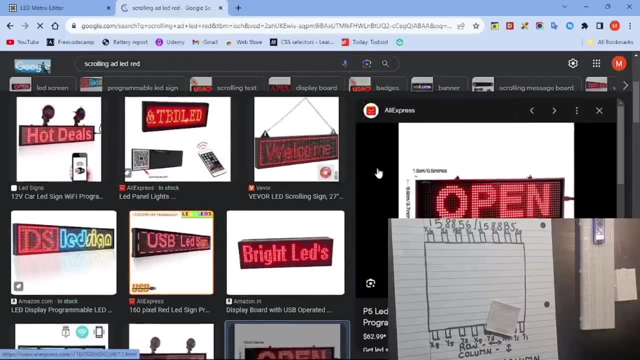 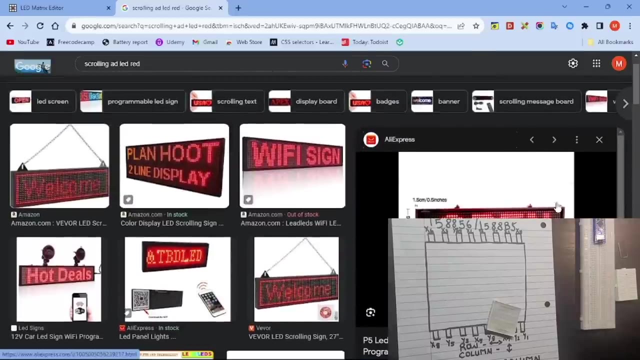 of you are very, very familiar with this. you these type of ads, and most of us see this type of these scrolling type of red leds, have you? you've seen lots of these led ads that scroll. okay, i think most of you have seen again these, again red scrolling led ads, and they're basically the same thing. obviously the the ones that are on the 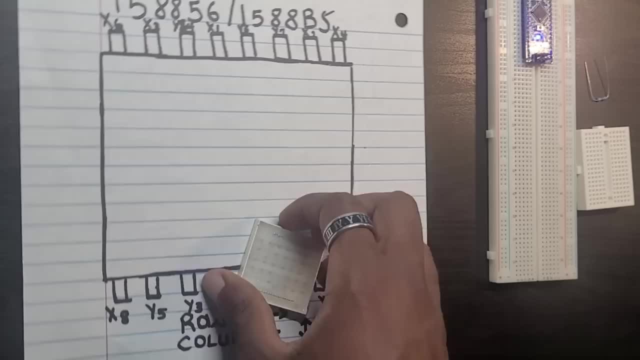 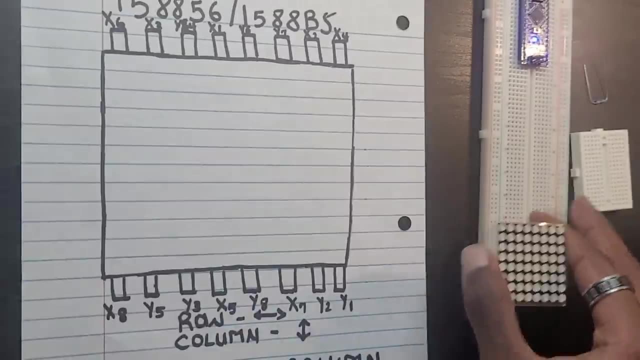 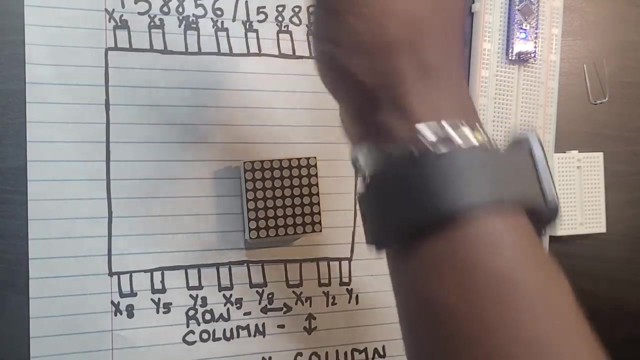 ads are obviously bigger and they're more capable, but they operate on the what, on the basics of this. okay, this is just that it's a very, very small one, okay, all right. so right here, why do we use led matrices, first things first, rather than these four digit, seven segment led displays? because we use this display again to display what we. 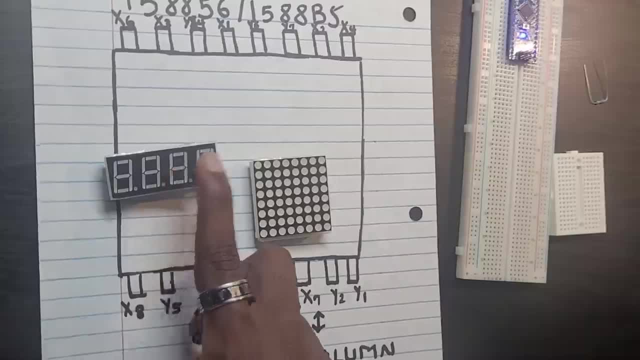 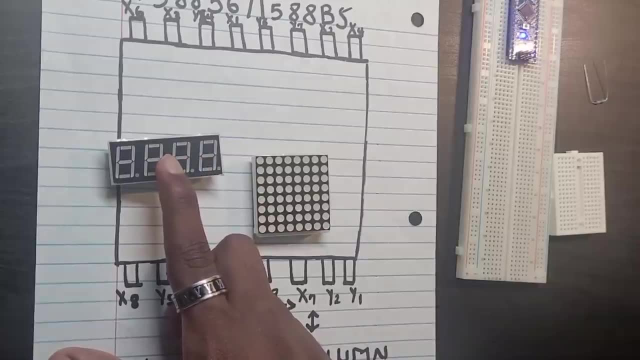 displayed numbers with it, any number that we wanted, from zero to nine, but obviously when you try to display, uh, something other than a number, for example an alphabet, we start running through. okay, so right here, let me just try to display small a. what should i even be turning on it's? 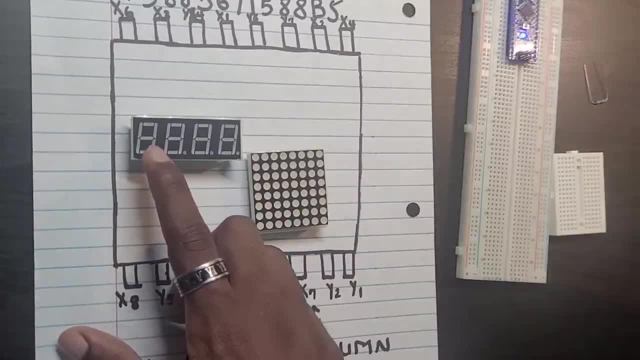 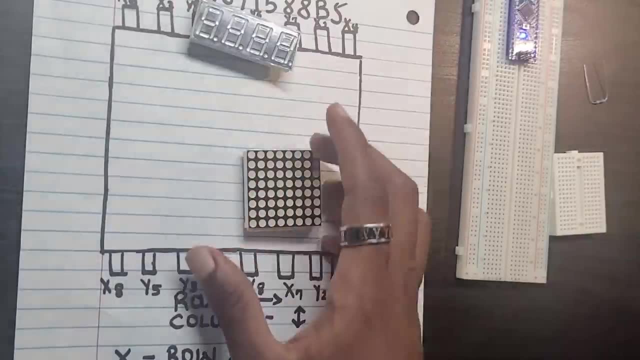 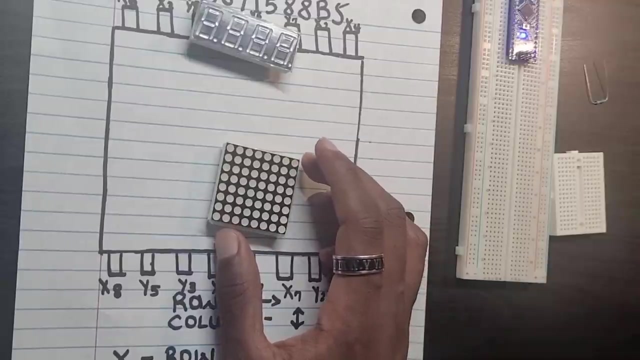 impossible to what. it's impossible to what. to turn on small a, for example, here. what to basically display a small letter, a? okay, but using an led matrix. what we're capable of, again, we're capable of what we're capable of displaying any type of alphabet, all right, small letter, capital letter. 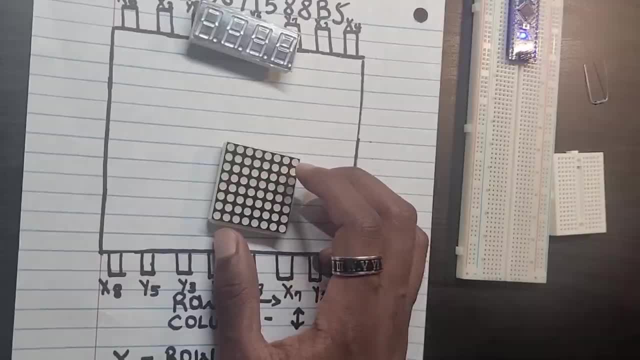 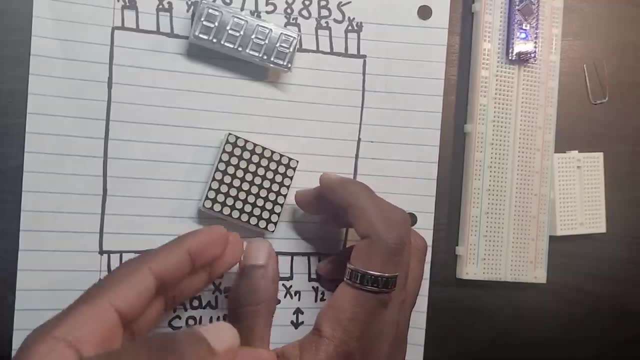 any number and even small, small types of images. basically, we cannot display a sophisticated image using this, but we can display simple images, for example, a smiley face, a frowny face and other than that. so we're going to display a little bit of what smiley again. again, we can display what. 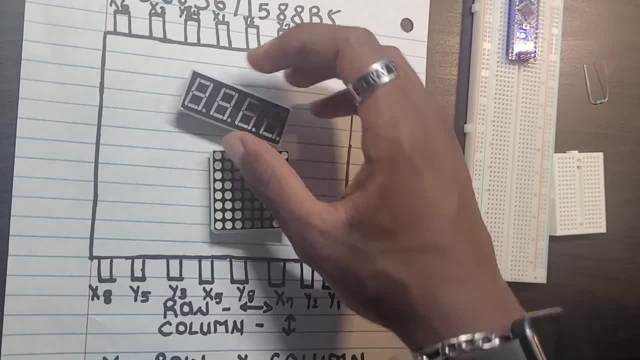 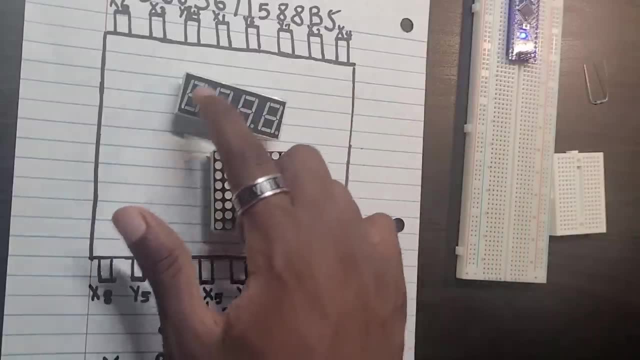 simple images, okay. so led matrices are more capable than what. they're more capable than our four digit, again seven segment led display. we use this again when we want to what we want, to only display what numbers. obviously they're no match to, obviously they're no match to our, again, lcd. 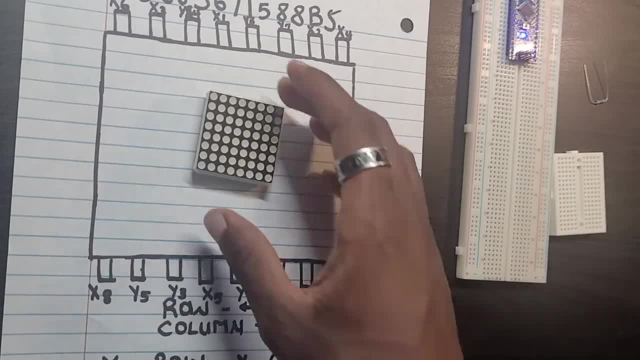 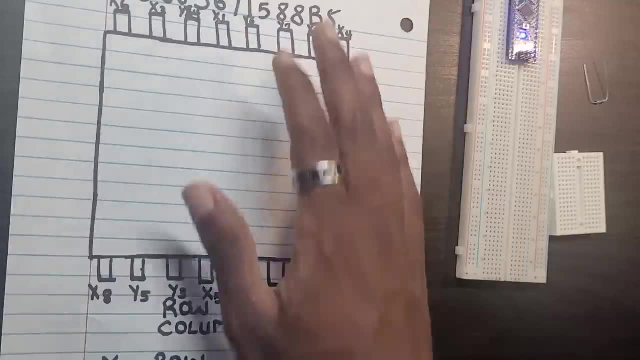 screen that we have on our phones and tablets and laptops, but they're way cheap and again, they're going to show you the text when you need them, so okay, so they're very cheap and again, very, very useful, all right. so now let me just show you how an led matrix works. 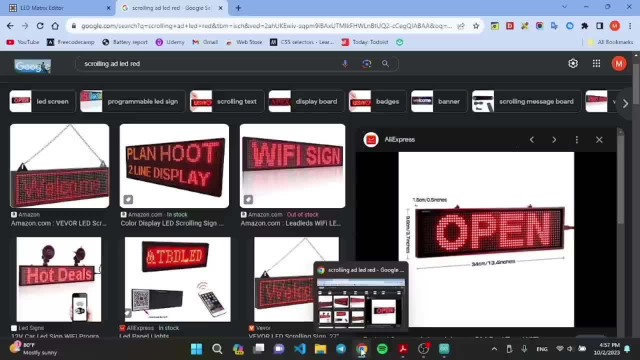 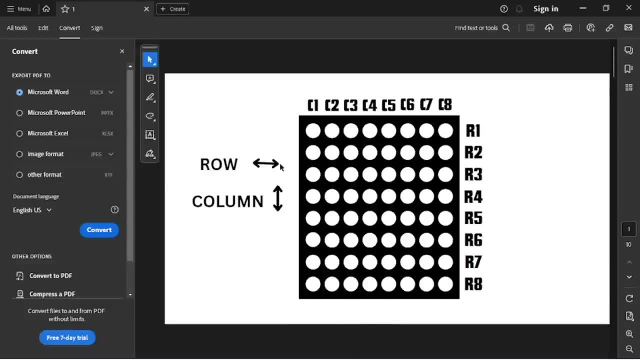 so, before even you know using it in our project, what we're going to do is check how led matrices work. okay, so let me go over to my presentation right here. so right here is what they're marked. every pin is marked with a what, with column one, column two, column three, all the way up to eight. 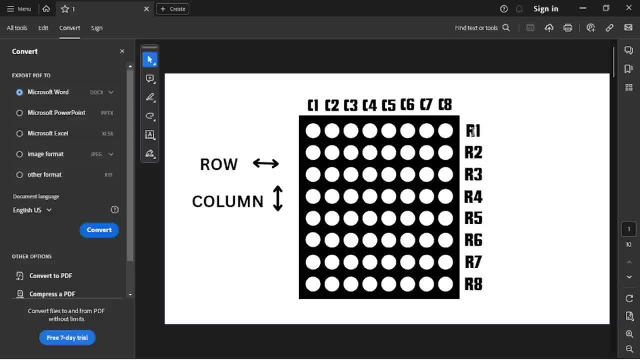 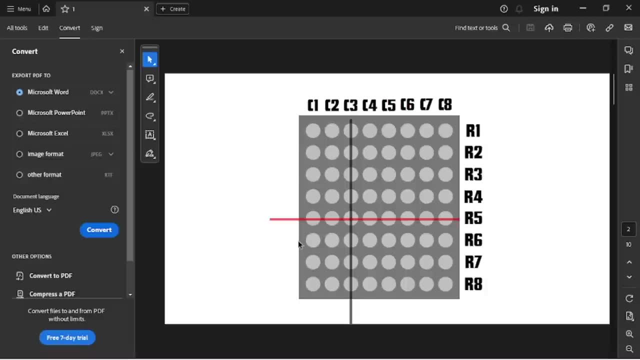 okay, the same goes for rows. they're what they're marked, from row one to row eight, and one thing i want you guys to understand is: row is what from left to right? extend this from left to right, while columns extend from what's from up to down. okay, so if you go inside of an led matrix, what you're 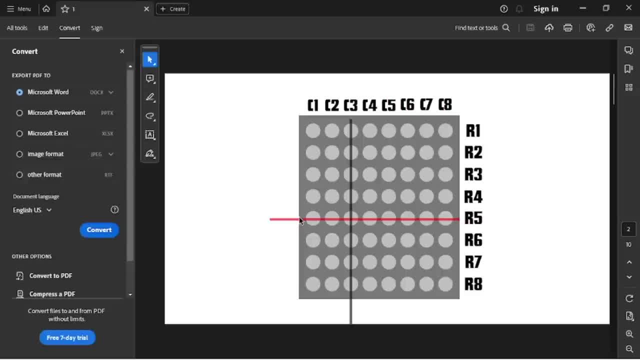 going to be seeing is what you're going to be seeing: lots and lots of wires. let me just show you a wire right here. this is basically the inside of what an led matrix you can see, what you can see. the lines here, the ones that again extend, the wires that extend from left to right, are what 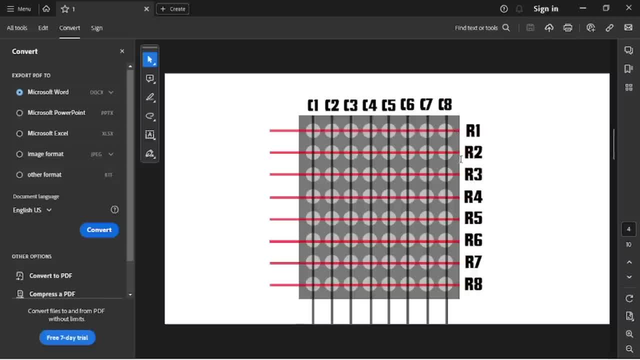 they're rows, okay, they're going to be these lines again. so i just want you to think of them as a grid. okay, they're going to be basically, what a grid, a grid of, what a grid of literally wires. okay, so you can see this again. they go to the corresponding number of rows. go from left. 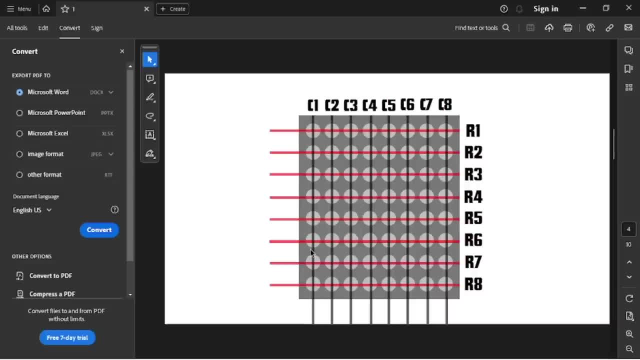 to right and there's columns marked with a what, marked with a black color. the black line is what columns and the red line is rows. okay, so how do we turn on the led matrix? so let me just show you on a specific, specific, what a specific dot, basically a specific led inside of this led. 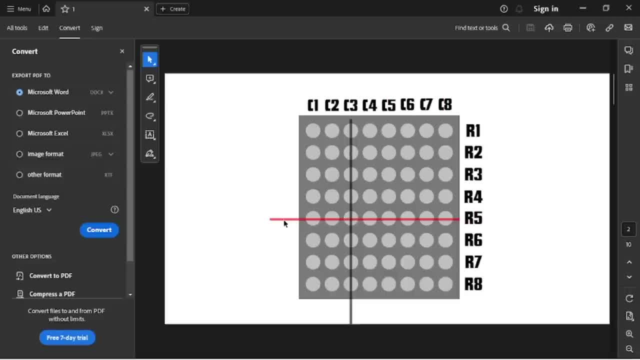 matrix. how do we do that? basically, what we do is: okay, we turn on r5, we set it to what, we set it to high. okay, we're going to be setting up- let's say, for example, we're going to be setting up r5 to high, row 5 to high, and then what we're going to do is what? set column 3 to low. when we do that, 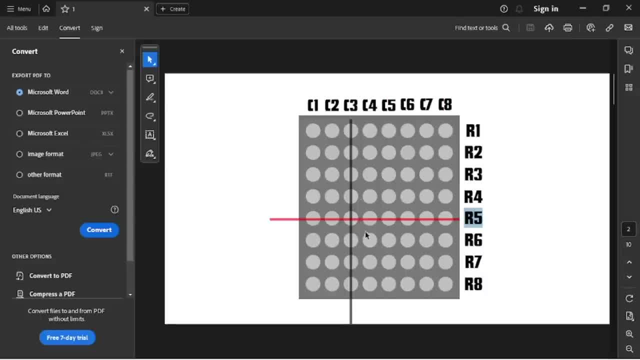 guess what happens. i want you to take a guess: which led segment lights up? is it this one specifically? or even: uh, the whole row lights up here. the whole row lights up. what happens, guys? just want you to take a guess. for those of you who guessed that: 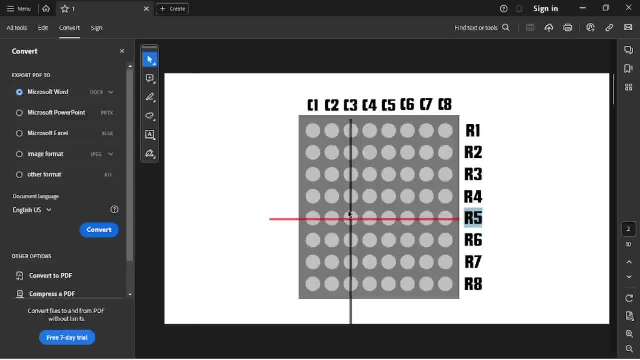 the whole row will light up. you're wrong, because what happens here is what the five volt is going to be connected. for example, let's say, to this led, right here, the led segment that's here. but the problem is what? it's not a complete circuit. a complete circuit always has what. it has what 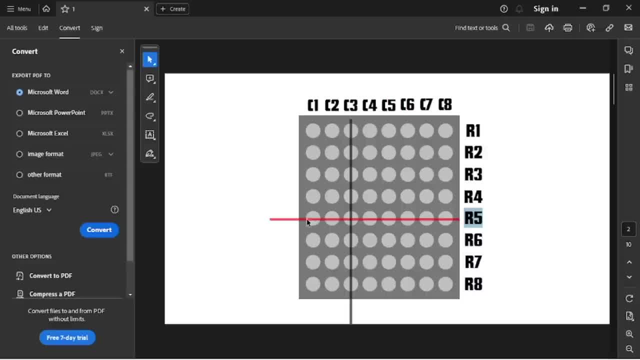 the positive terminal and the negative terminal. okay, so in this case it has the five volt again, but it does not have. what a negative terminal. so, specifically here, it's not going to light up. the same goes for this one, for these ones that are here, but when it comes to the one that is again, 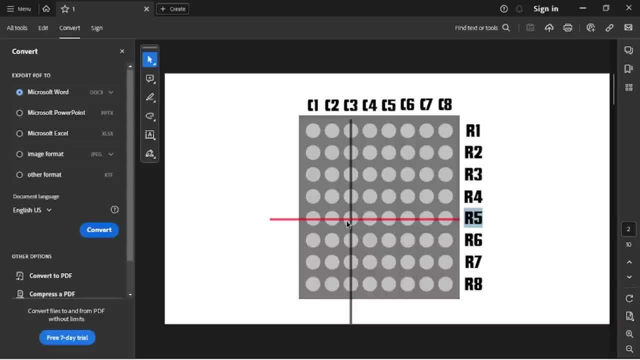 located at row five and column three. what happens is what? what happens is what it lights up, because why we have the five volt coming in from row five and we have the ground pin, the negative terminal, coming from what? from the column three. so it's going to what it's going to light up. there we go, it's going to light up, okay. 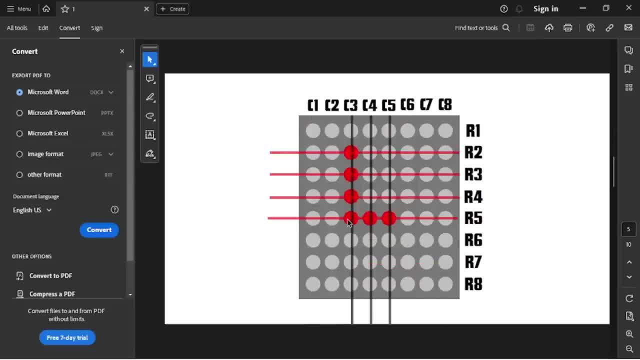 that's one thing i want you to keep in mind, all right, so let's just move forward right here and let's try to draw an l. okay, let's try to draw a simple l? um. one thing i want you guys to actually keep in mind when trying to draw these simple else's: what do we need to turn on? 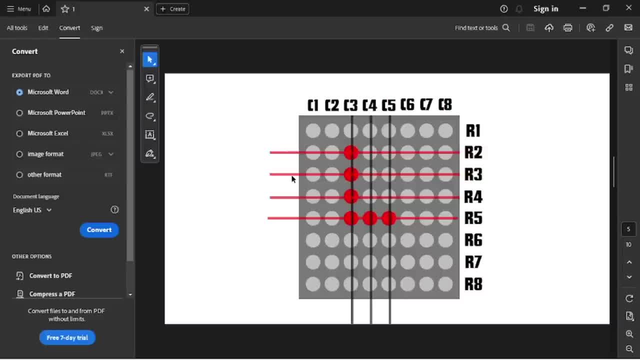 we need to turn on r2? okay. we need to set r3 to high, we need to set r4 to high? okay. then we set r5 to high. and then, when it comes to the columns, what happens? we turn on c3 to what we said, we turned it on to low. so basically what we create a full circuit for these four leds. 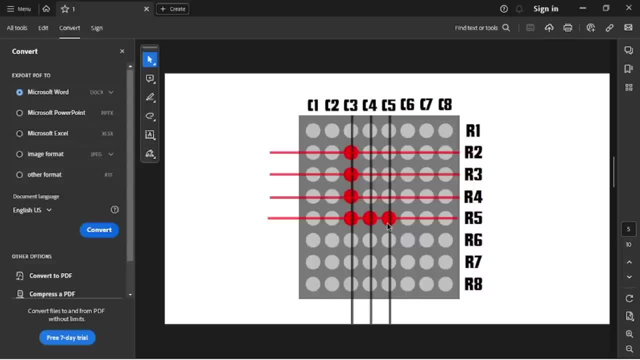 and then we set c4 to low and then c5 to low. i think most of you would suggest me to do what? to do this? to get what? an l? but there is a problem here. okay, and this is literally what. this is the result that we expect, but what actually happens is what actually happens. is it's going to? 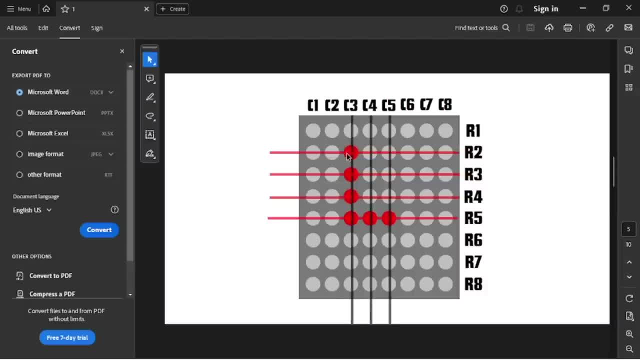 light up like this. why is that so right here, unintentionally, unintentionally, we lit up what column four and row two. row three and row four are already set to what they're already set to high because of what we're again talking about? what column three? but we already set column four to. 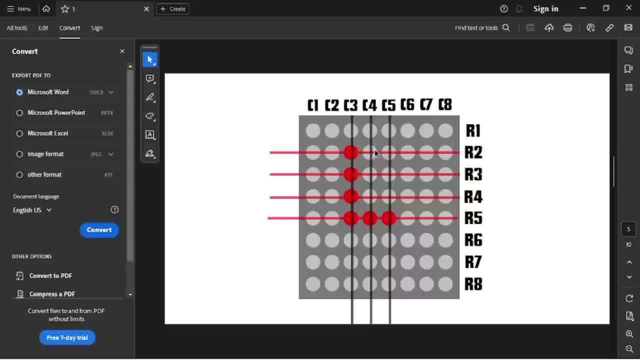 low. so basically, when they intersect right here, basically what, we're gonna have a full circuit. so when you have full circuit, what happens in this case? it's gonna what it's gonna light up. so these are the light up, and the same goes for what c5. so it was more of like the problem that we had. 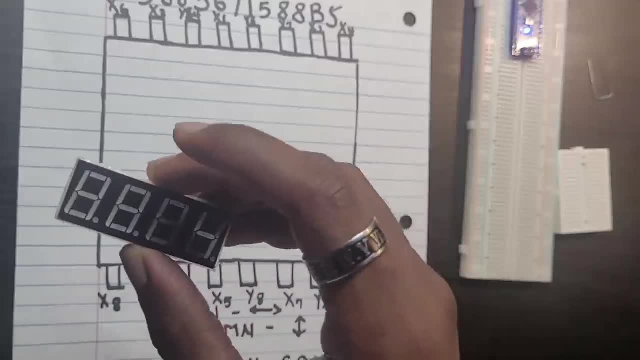 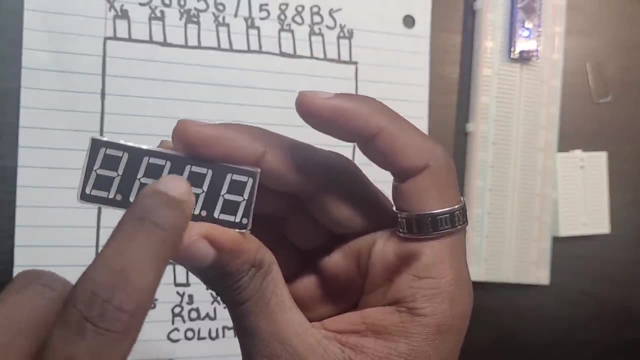 when we were working with the four digit for the four digit, uh, seven segment led displays you remember we did was what: we tried to turn on everything right here. we tried to turn on four of the digits right here. when we tried to do that, it started what started: copying the first digit. 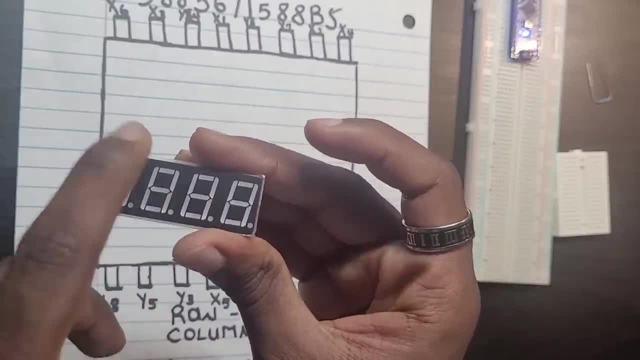 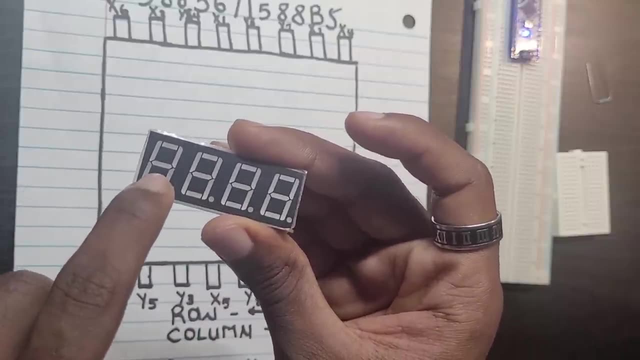 and the first just started copying the second one, and the second one copied the third one, and third one copied the fourth one, basically giving us the same thing. so, for example, if i turn on seven right here and try to turn on all of this, four digits at once, where we? what are we? 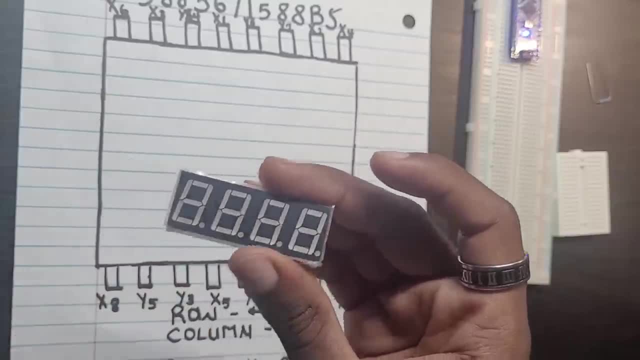 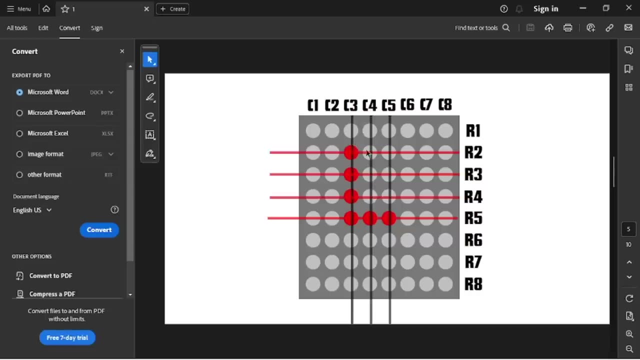 going to be getting. we're going to be getting seven, seven, seven, seven. okay, that's what. that's what basically is happening. so if you look right here again, what happened is what the column four, what started to copy column three. that's what's going on. column four copied column three and 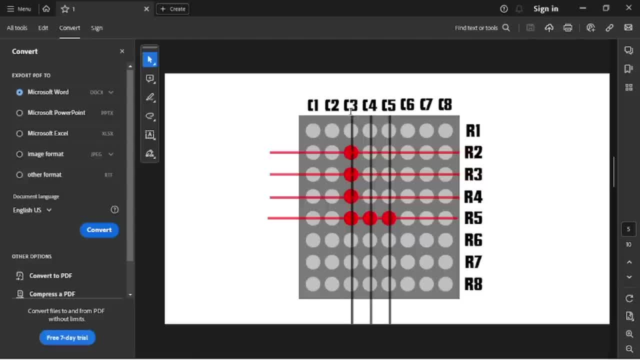 column uh, column again five copied column three. can you see that? what happens is there, we go it started to copy it and basically they're literally what they're literally the same. right now, column three cover four and column five light up the same, okay. so how do we prevent this? 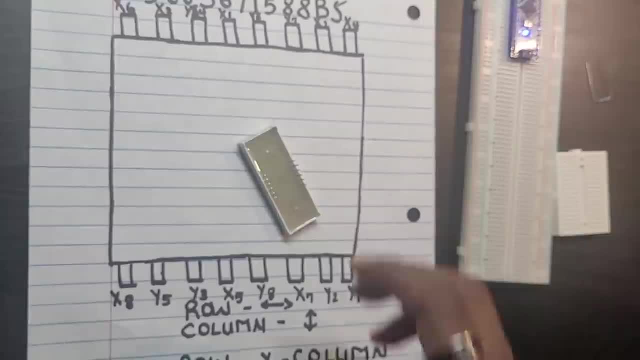 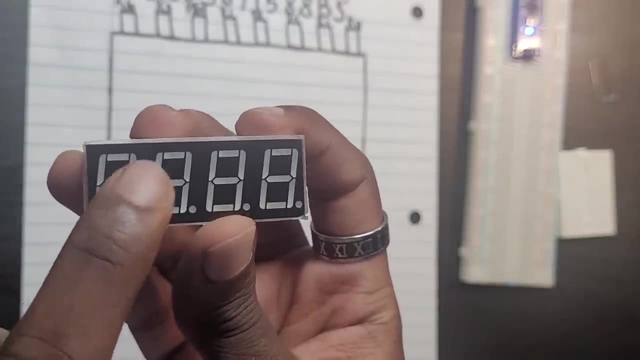 we do the exactly what we just did when it came to what? when it came to the four segment? uh sorry, four digits, seven segment led display, what did we do? we only displayed one digit at a time, and then we switched from one digit to another digit, right. so, for example, right here, i displayed 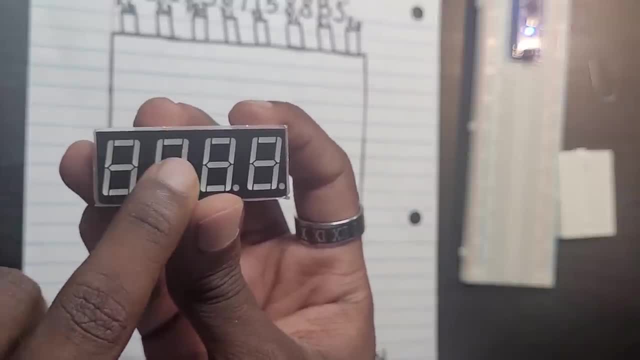 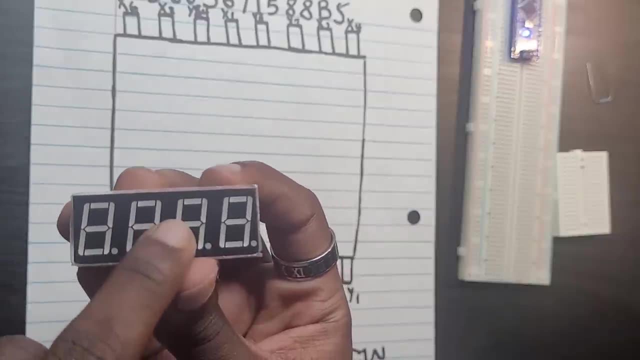 eight. and then what did i do? i moved to what i moved to here and then displayed another number, for example, let's say two, and then, after i'm done with that, i don't know what i'm going to do now. i'm just playing what? let's say three, right here, and then i'm done once i'm done with this. i just played. 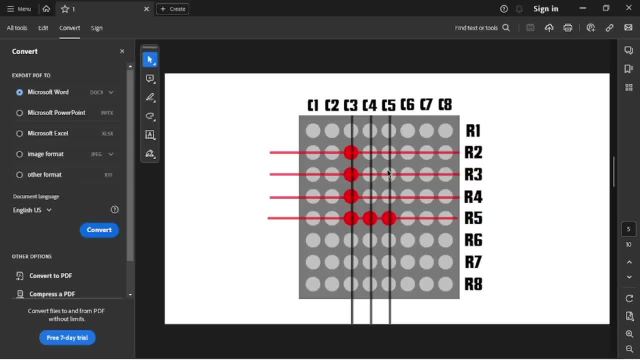 four. but again one thing: obviously arduino did so good as well. it was very, very fast. the arduino was very, very fast at scanning and again going, turning off the first digit, going to the second digit. it was so fast that for our eyes we can see all of them is on. so basically, what we cannot see, 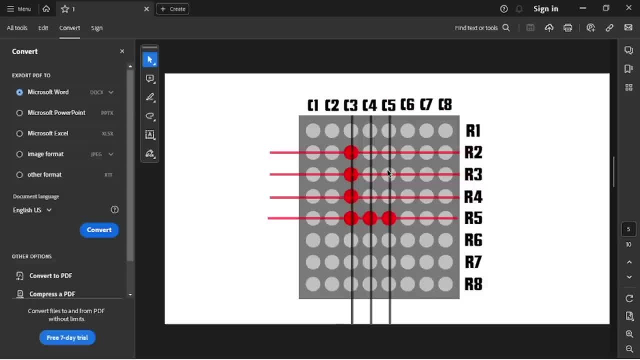 arduino physically doing work. arduino turning off the first digit and going to the second digit. it was that fast, so we're going to be doing exactly the same thing here. so what we're going to be doing is what? okay, we don't want to get column four and 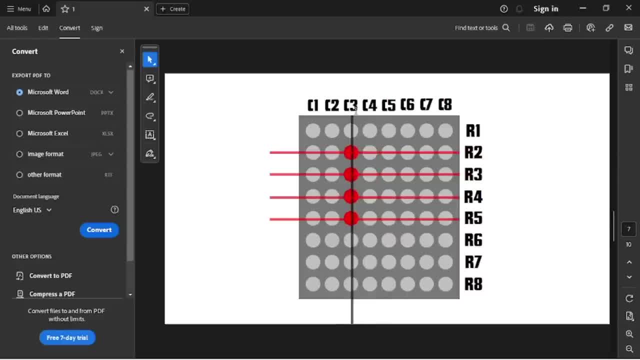 column five to copy what column three. so we do, what do we do? we only turn on column three right here. okay, one part of the l, we're trying to again, uh, write down capital letter l. what we're going to do is what: we're going to set up r2 up to r5, to high, and then we're going to set column three to 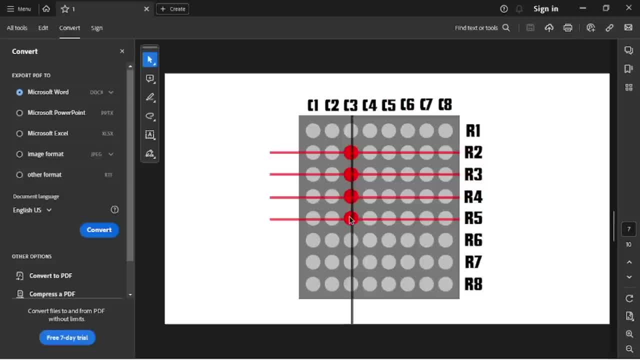 low. so we're going to basically have what this line. once we do have that, we're going to what we're going to automatically, what we're going to turn off what column three? okay, we're going to be turning all of them off, okay, so we're going to be turning this to what we're going to be turning. 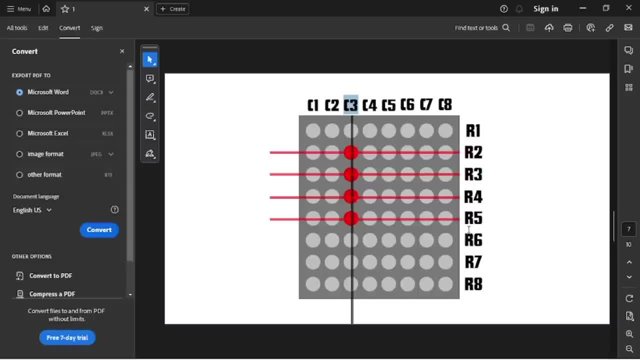 column three to high, and then what row two up to row five are going to be, what row two out to row five are going to be set to low then afterwards, what do we do then? afterwards we, what we focus on, what we're going to be turning on row five and then we're going to be turning off what we're. 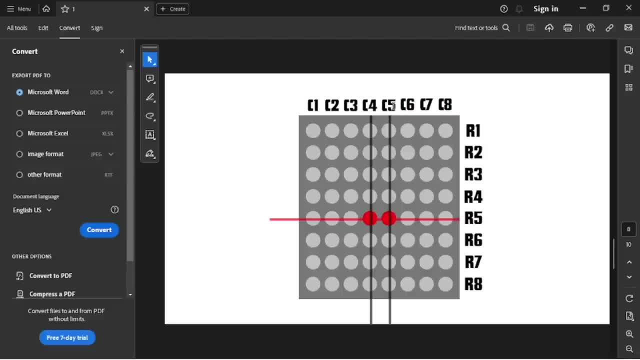 going to be setting this to low and we're going to be setting this to low column four and comma five. so basically we have one, we have an l. obviously we cannot see it right now as if i'm just doing it, but if i even try to use this on the presentation, let me try to actually toggle between it very fast. 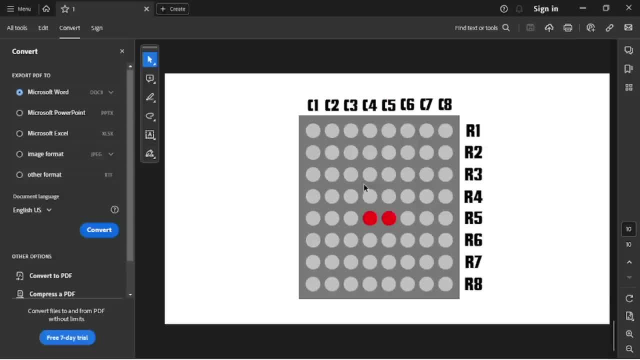 so you can see it. okay, so you can see somewhat of an l right here. obviously i'm not doing it as fast as the arduino. when the arduino does it, it's going to be so seamlessly fast that we're not going to be noticing it. but even right here you can notice a flickering l. okay, you can notice a flickering l. 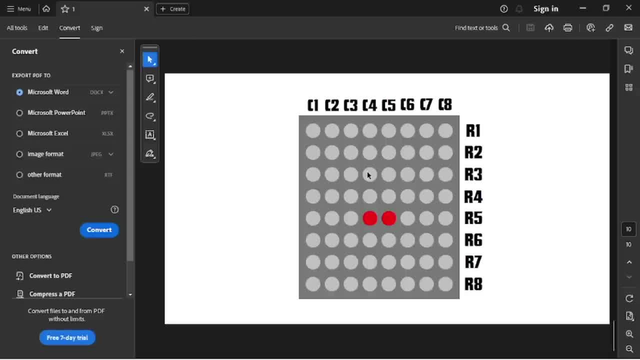 so, basically, i'm going to be doing this right now, and i'm going to be doing this right now and i'm arduino is going to do it really, really fast and what, so that we cannot notice it. okay, one thing again i want you guys to keep in mind right here is what the difference in the model? there are lots. 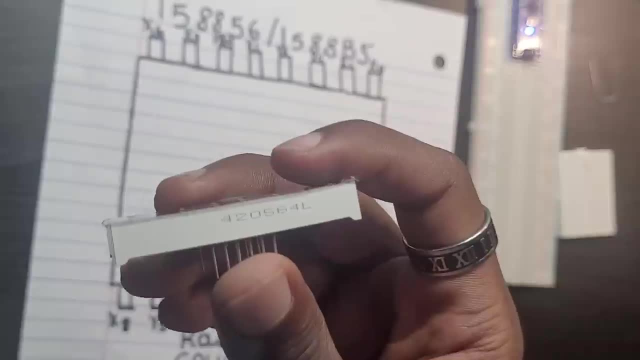 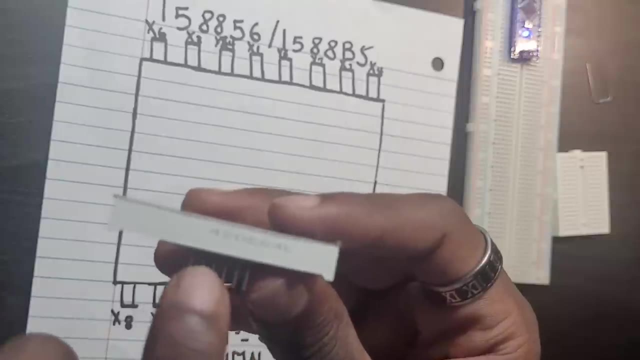 of again, difference in models when it came to the four segment uh led displays, the four digit seven segment led displays. obviously the pin placement is going to be what? different according to what, according to the number you have. again, what i want you to do is what? find the corresponding number? 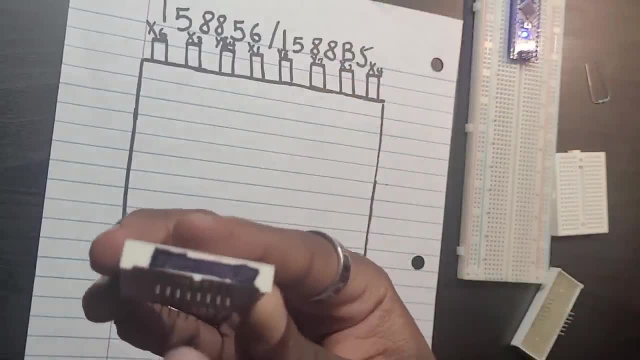 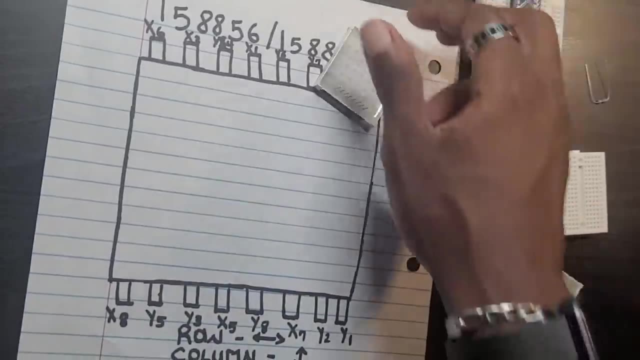 in your led matrix. i want you to find the corresponding number and then do what? and then google the data sheet. if you don't have your data sheet, you're going to be doing exactly what i just did for the one for the four digit, seven segment led display: we're going to keep on trying to turn. 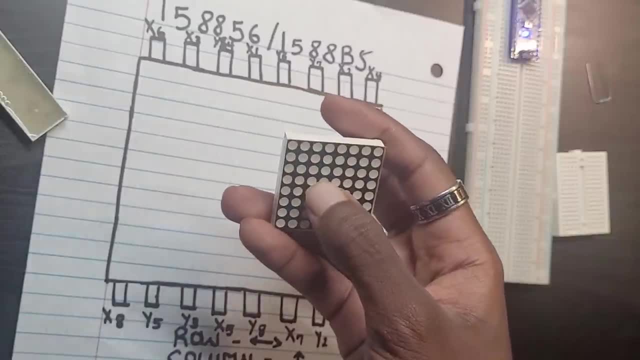 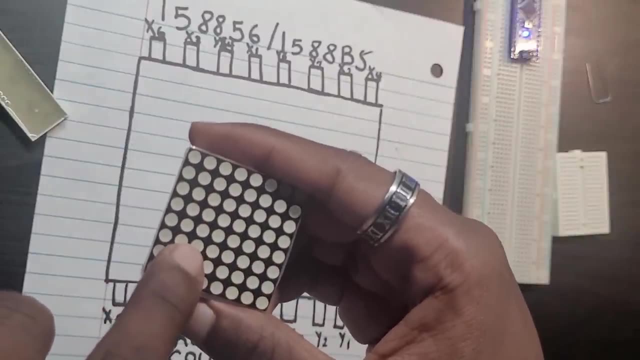 on one segment right here, one light as soon as we do, we're going to be extracting what. we're going to be extracting information right here. let's say this one lights up in this case: okay, let's say this one lights up. i'm going to say this is what i'm, this is going to be what row six and it's going 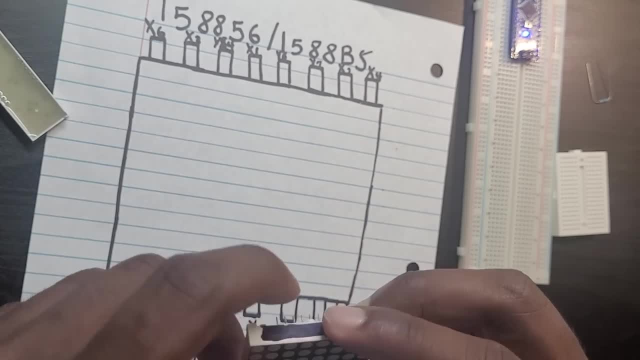 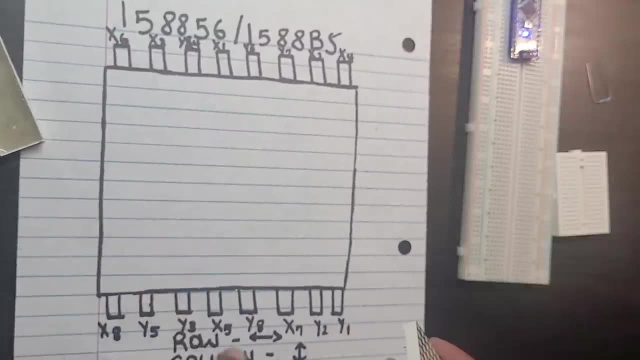 to be column three and i'm going to be extracting the information right here and i'm going to be again talking about the corresponding again pins that i get attached and obviously, what do i need to do afterwards? i can extract information and create a data sheet myself, okay, but one thing i 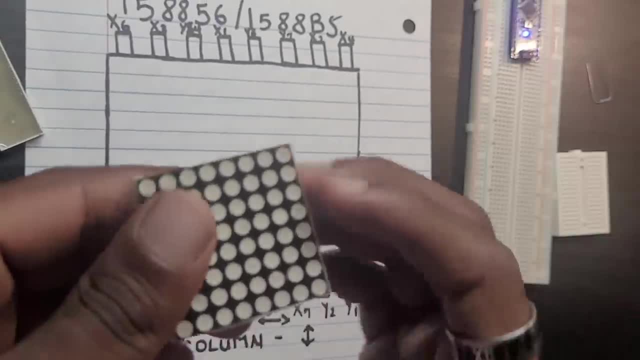 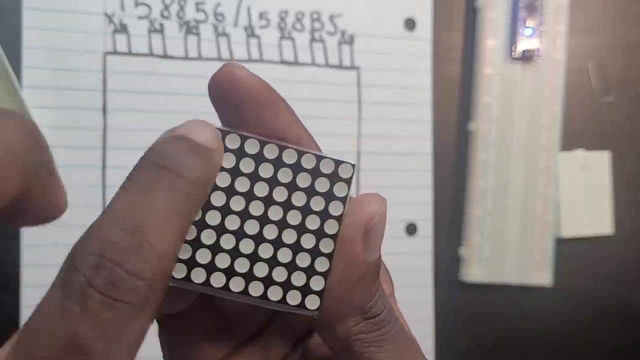 want you guys to keep in mind is: okay, right here, i can just say this is row and column. okay, i can just flip it again and say this is row or column. i can just say this is again. this is row, this is column. i can just say: this is what. this is row, this is column. so one thing i want you to get: 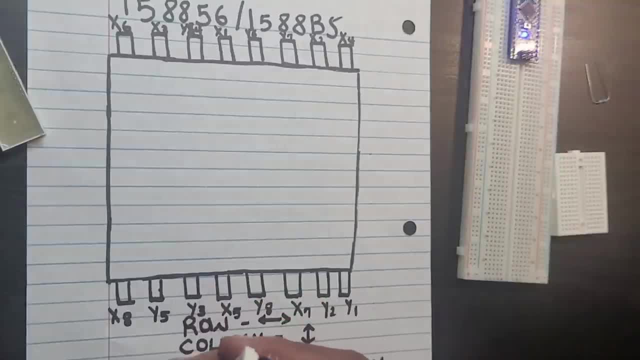 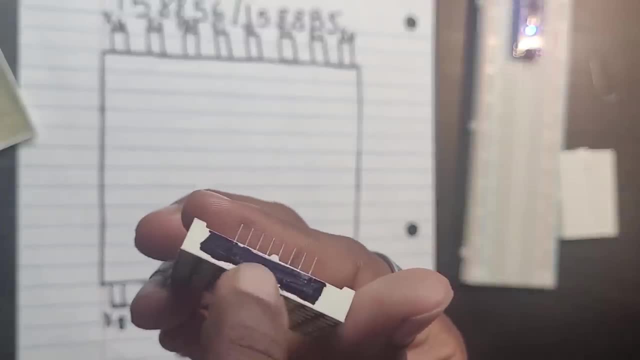 to always, um, to always keep in mind is okay. i want you to put the one that has a number right here. it is faded. what happened to mine was it has faded, so i just put a black sign on it, okay, so to just indicate which direction is. 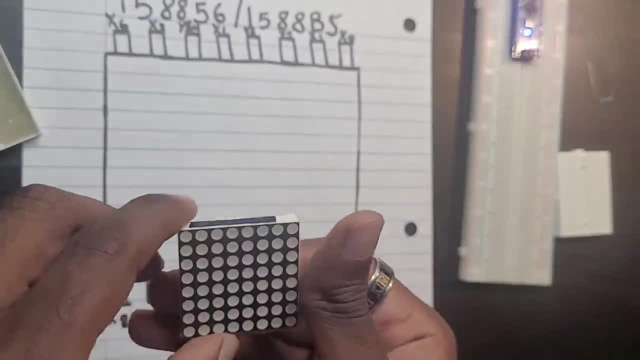 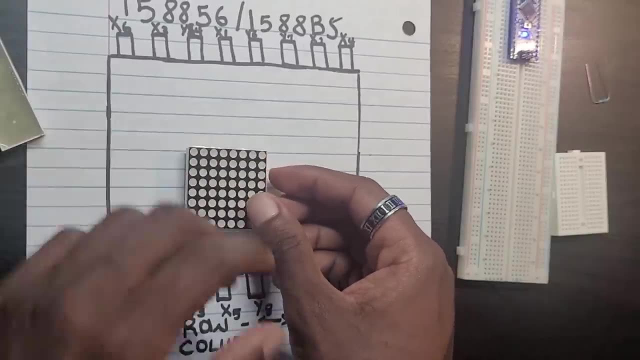 which. so one thing i want you to always keep in mind is the pinheads are supposed to be like this. when they're on the opposite- okay, and again the one that has a number, it's going to be placed like this. it's going to be again placed what like this, and then you can write down your pins. okay, so i 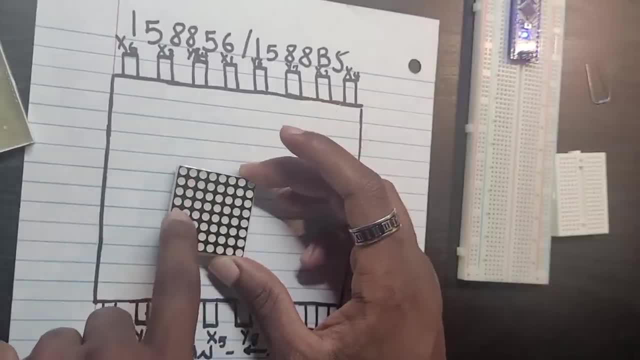 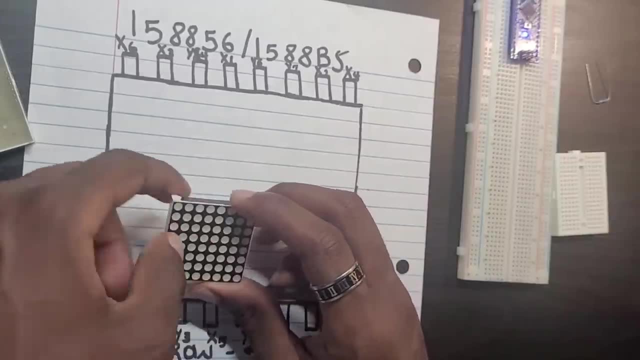 want you to write down your pins like this. so this is going to be what: when you talk about row one, row two, like this, you're going to be keep on talking them, like how you're going to be placing them like this. this is very, very important. okay, if you just do that, you're going to be interchanging. 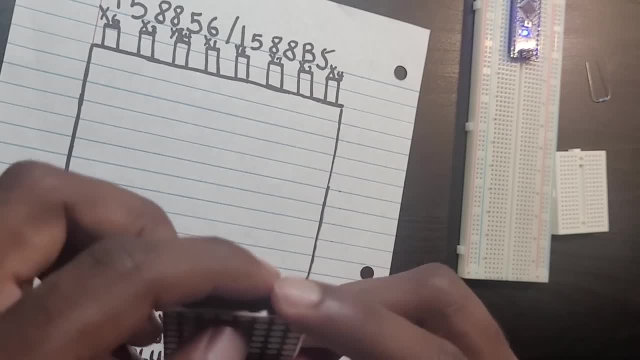 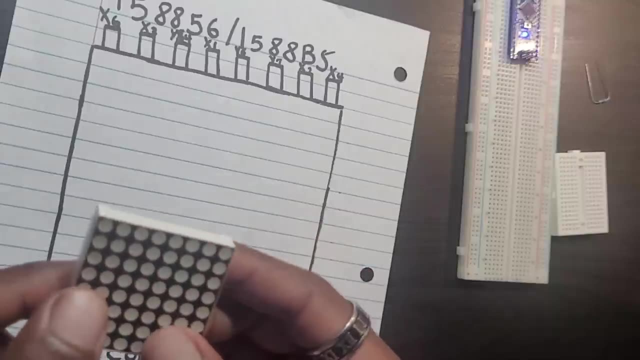 if you just, let's say, not use this one, where the pinheads are like up and top, top and bottom, and if you just place them left to the right. when you place them left and right, what happens is what? the row is like this, and then, well, we just interchange the row and the column. they basically what they. 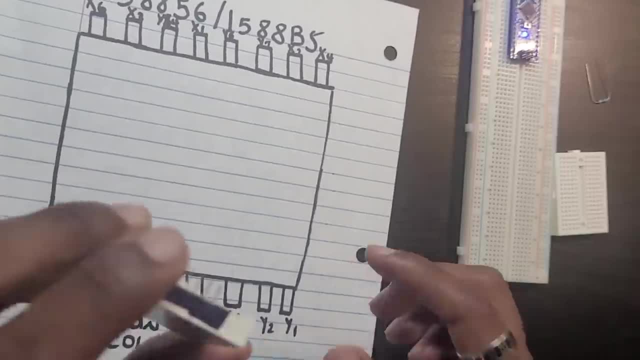 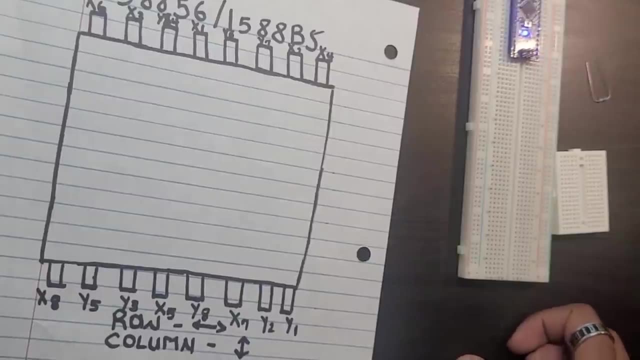 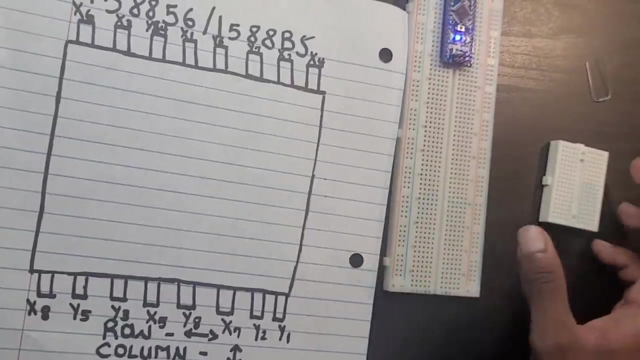 basically switch. okay, so just keep that in mind. so always keep them from top to bottom okay when with them okay. so, with that being said, before, uh, we actually work in our first project. let me just try to, uh, light up one led segment right here. okay, so i get my led again, and because the led 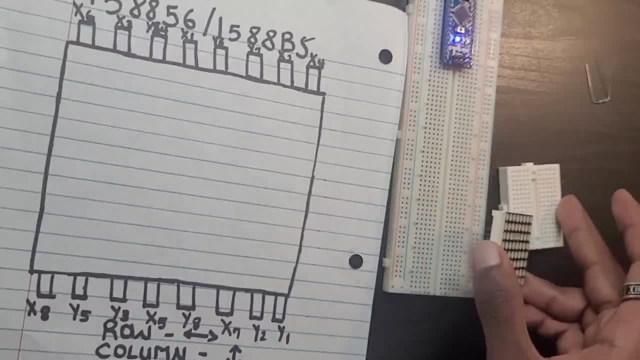 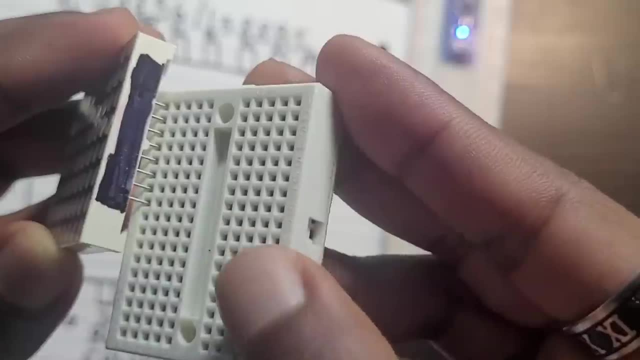 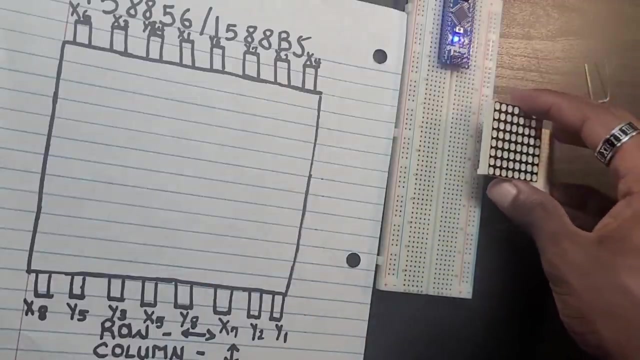 takes a lot of space. i'm going to be using a separate breadboard right here. to make my life way easier, let me just connect that breadboard, the led, first. hopefully you can see it there. we go, connect it in such a way and then connect this right here around here. okay, i'm gonna need my 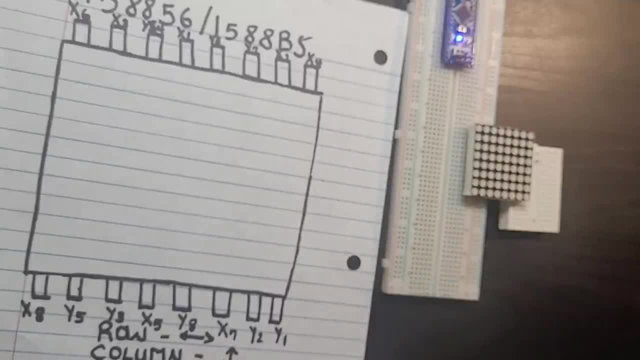 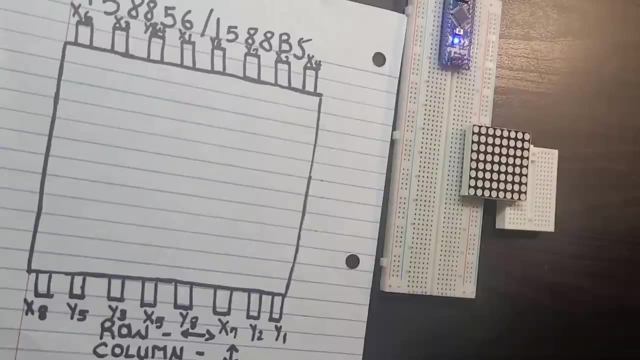 resistor right here. obviously i need my resistor. i just want you to think of them as what is leds? i just connected an led directly to what? five volt, and the gnd. what happens to it? it's gonna what. it's gonna be fried. if i brought my normal leds right here, if i had one, there we go. if i. 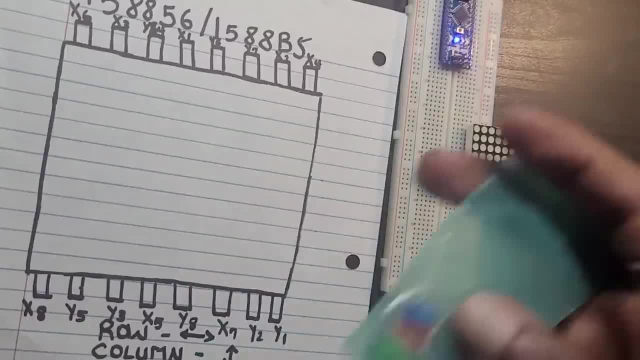 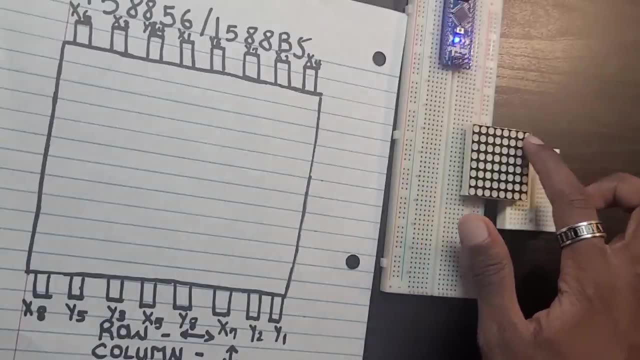 brought my normal leds right here and just again connect it here, and then connect it here, and then five volt and gnd. what happens? it's gonna what? it's gonna be fried. so i want you to think of them as what? as leds right here. we have 64 dots right here. i just want you to think of them as 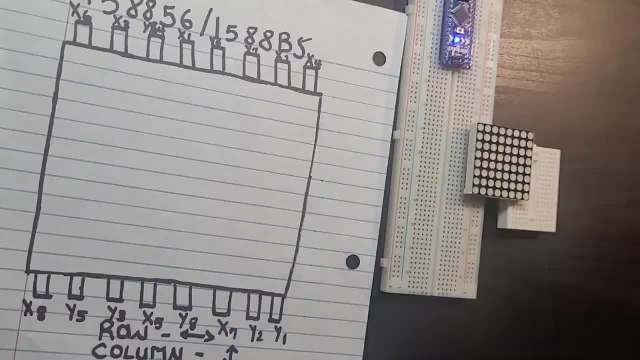 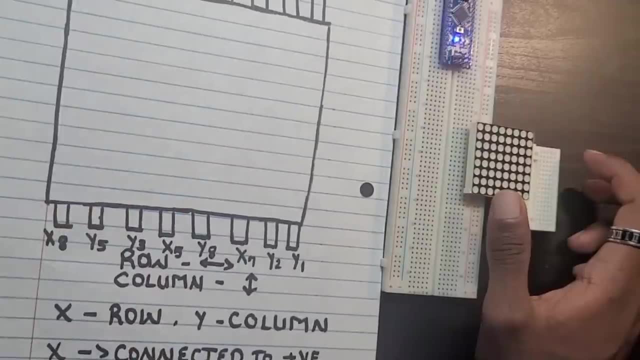 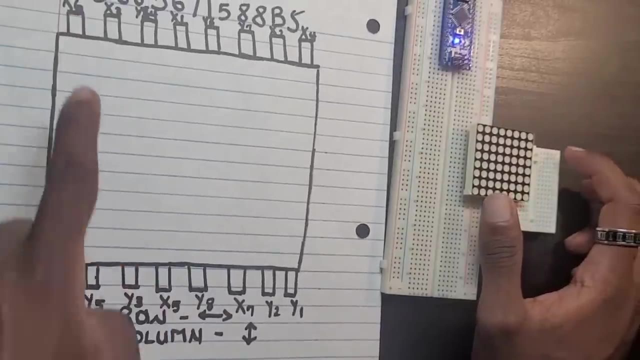 64 leds okay. so right here, what i'm gonna do is put a resistors resistor right here. there's a documentation right here. x indicates okay, x indicates row, y indicates column. this is my documentation, my version of the documentation. so i want, let's say i want- to turn on x6. okay, i'm. 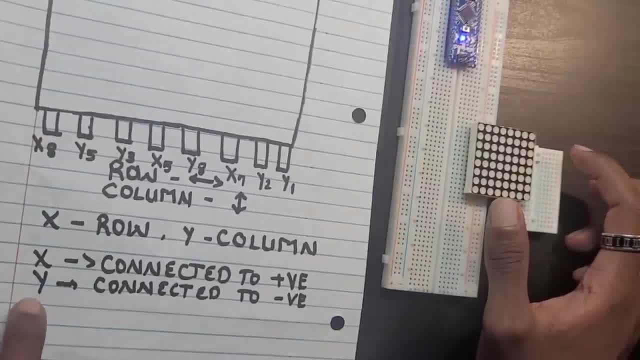 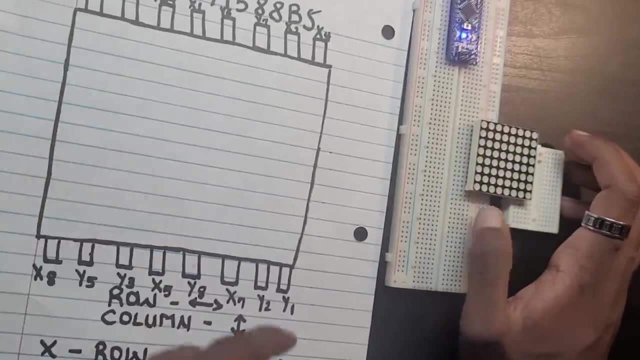 going to be connecting it to what. i'm going to be connecting to the positive, while y is going to be connected to negative. okay, so let me just do that x6. which one is going to be x6? x6 is going to be the one that is marked with a what that has a number, for you most likely has a number. 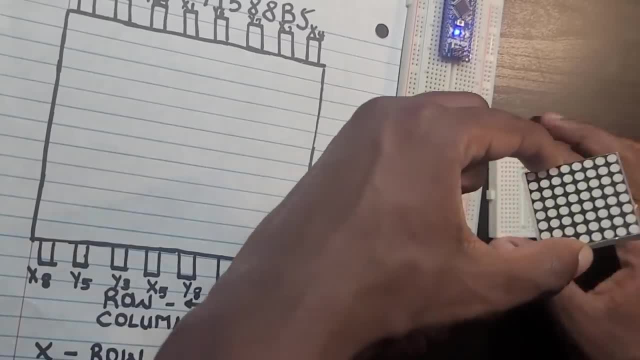 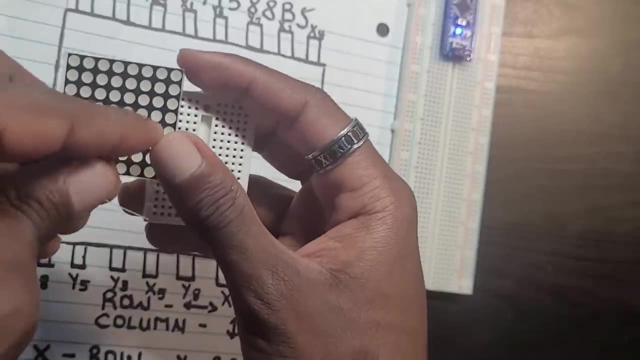 mine has faded, so i just put a black sign on it. so right here, let me just put it back again. i just remove this so i can show it to you guys. let me put my resistance right here. let me just make sure that it goes across, because i don't want it to touch the 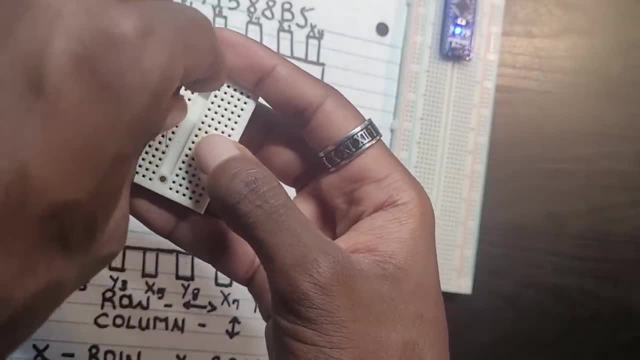 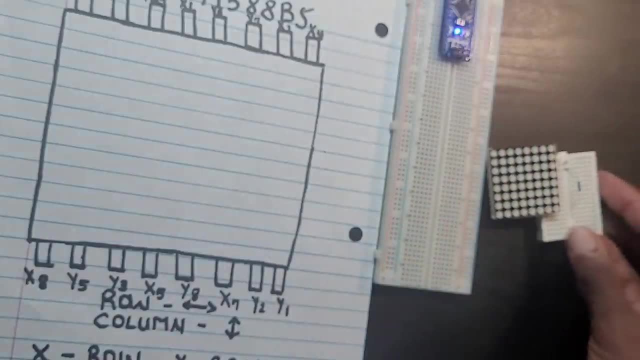 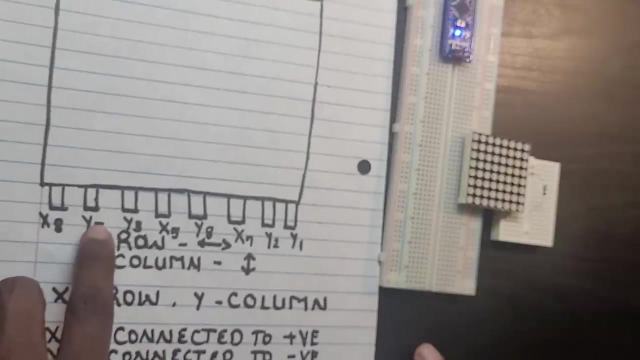 you don't want it to touch the the other led pins right here and then just do that. okay, that seems good enough for me. then afterwards, what do i do? i need my gnd. i need to connect to one of the columns. right here, let me just go to column y5. right here, let me just go to y5. 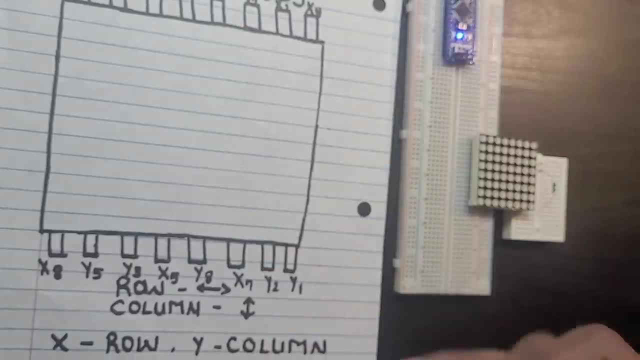 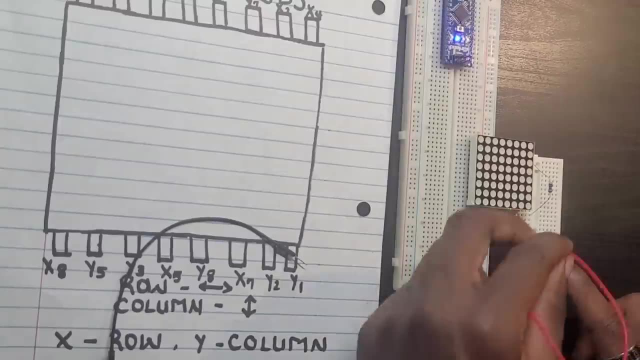 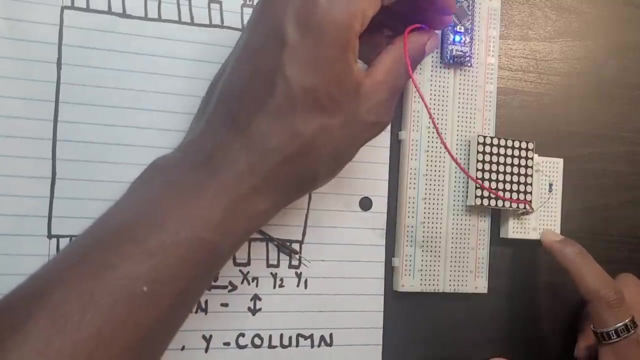 why not? let me just do that. let me bring two wires. let me bring a red wire, let me connect the red wire, let me just focus it right here. let me connect the red wire right here, the red wire to the 5 volt. all right, five volt right here, connected it to five volt, and then i'm going. 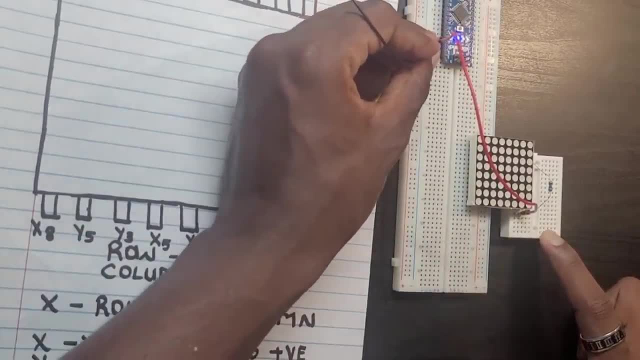 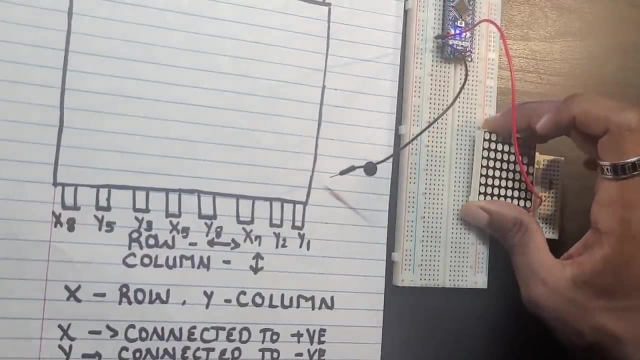 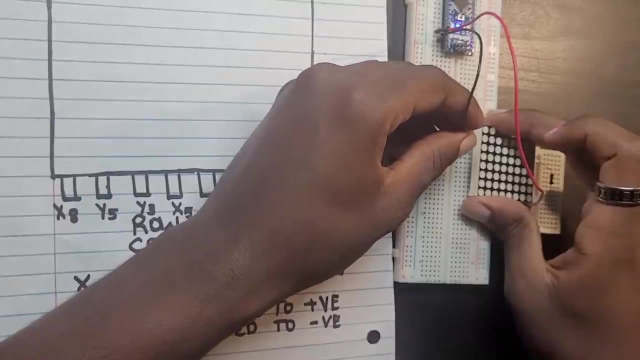 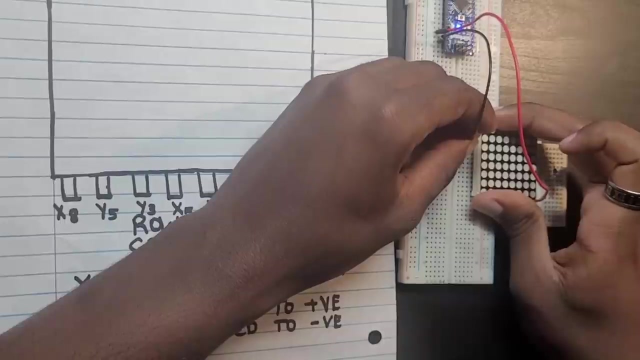 to be connecting my gnd. there's my gnd, my handy gnds here. there we go, and i'm going to be connecting it to the pin next to the very, very left. okay, i cannot see it from this angle because i don't have. let me just, it's very hard to see from this angle. wait, when I push it in, just, 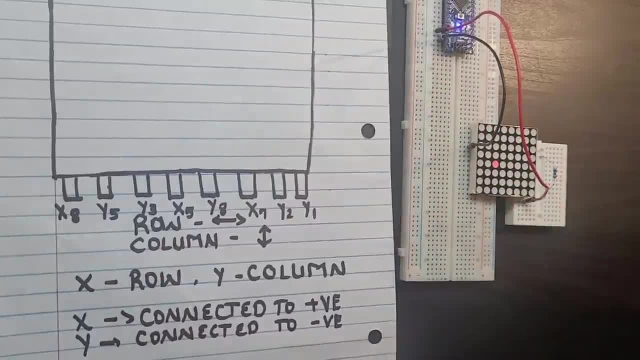 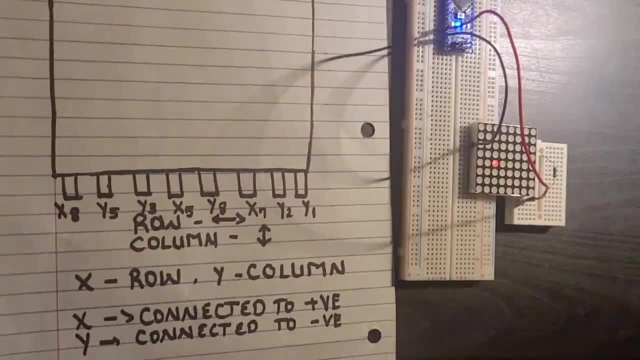 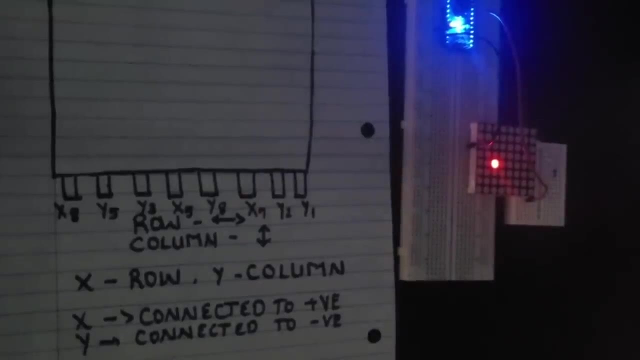 tap the. there we go. now it should be lighting up. there we go. I'm just turn off the light, turn off all the lights. so you can see it, there we go sliding up. nice, there we go sliding up. and let me just turn off the. turn on the. 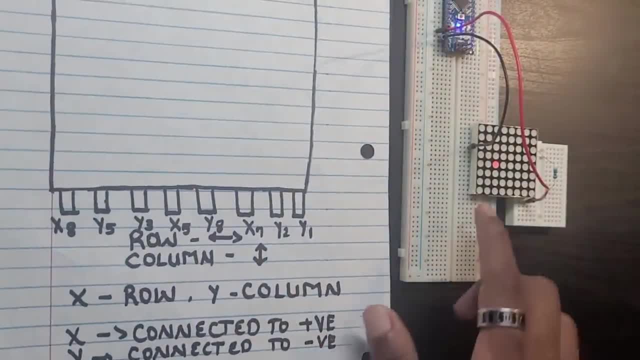 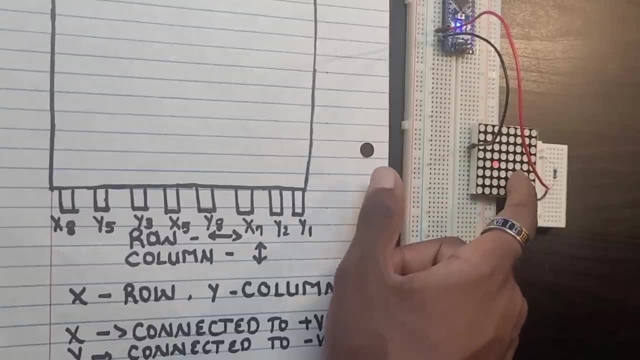 light back again. let me just do that. there we go, and one thing I want you guys to keep in mind is: what is this again? let's count all the way again to rose. if I count all the way, row three, row for row five, it's gonna be row six. 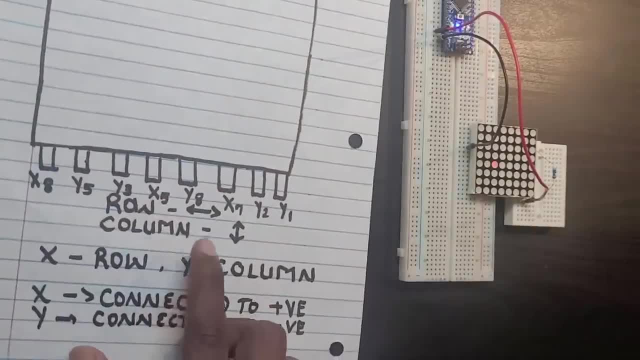 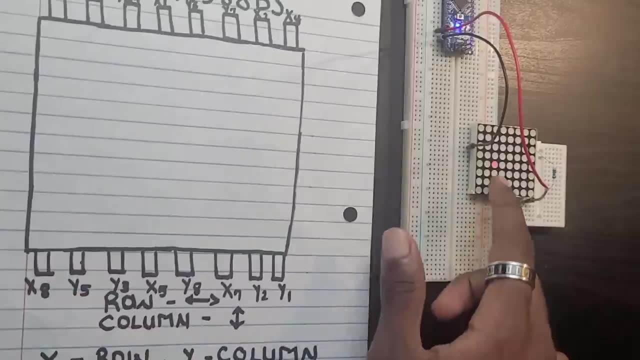 again, it's connected to what? to x 6, which means what x represents row, and I said so. basically, what x 6 is what row six? okay, it's connected to what? column five? all right, let me go to column. read it from up to bottom: one, two: 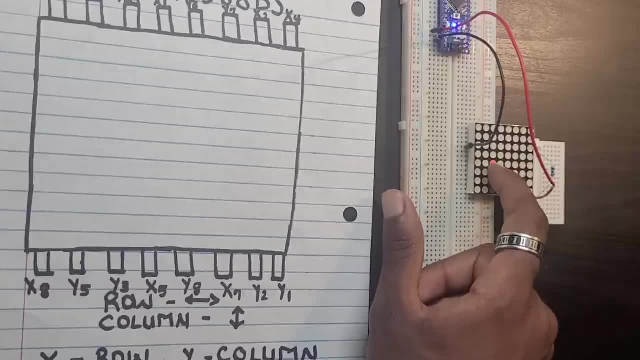 three, four and five. basically this is what y5. there we go. so it's connected to what column five and what row six. there we go, sliding up. but one thing i'm going to tell you guys is all right. one thing is this is how we're conventionally used to what lighting up our leds, we first put what. 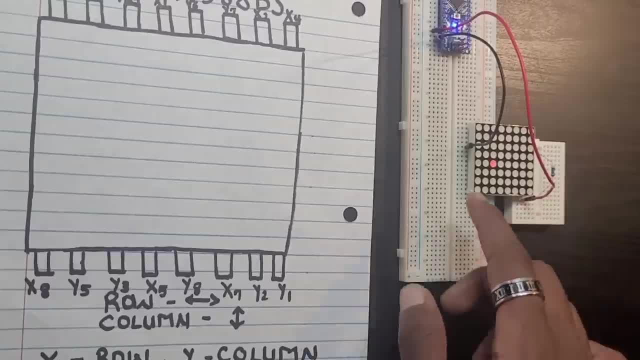 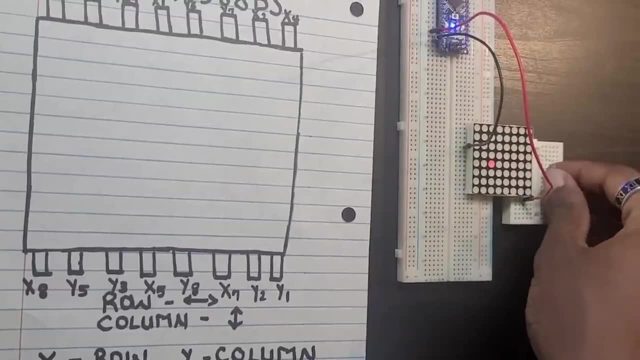 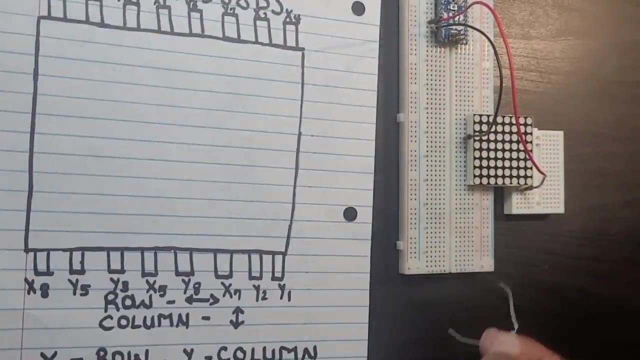 we first put our resistance and then put what? the five volt and then the gnd. but we can also do what. we can also do it another way. we're going to be putting our resistor instead of placing it on the gnd, right here. let me just unplug my arduino instead of what? using the resistor. 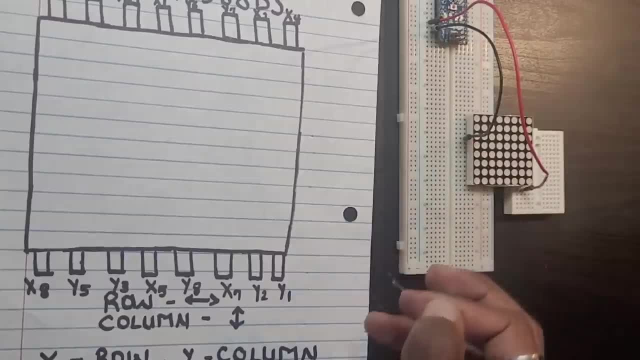 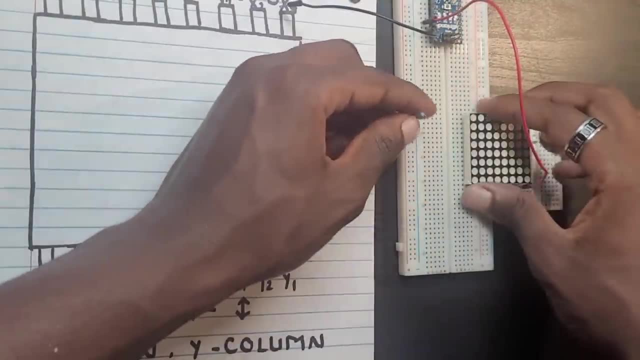 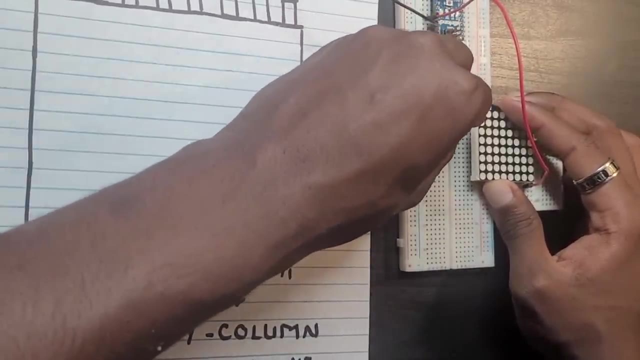 on the five volt. we can use it at the gnd, okay, so let me just do that. it's really hard to focus and film at the same time. why wiring it up is really the biggest problem when it comes to these led displays. wiring it up is literally 90 of the problem in my experience. okay, there we go. the resistor. 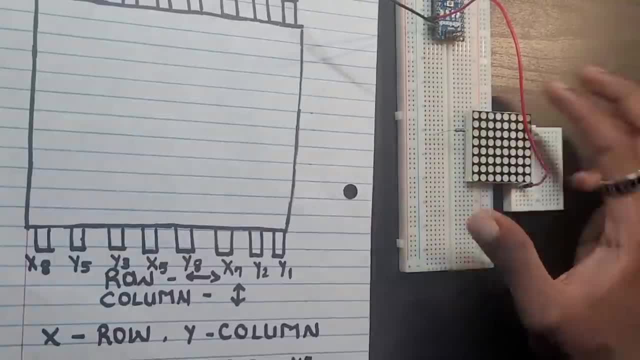 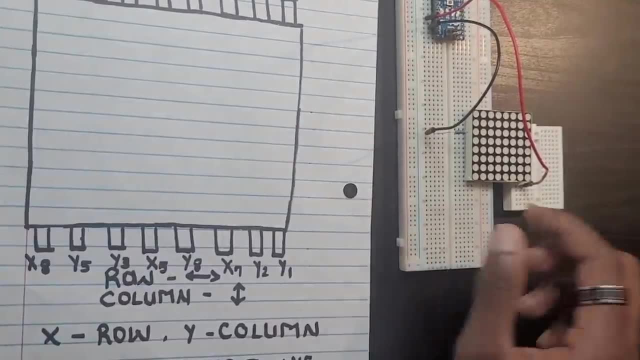 should be connected to the same. okay, there we go. i think it is all right, let me just do that. and there's our handy gnd connected to that one, and the resistor is going to be what to the gnd instead of what, instead of being to the five volt. let me put the five volt back to its place. 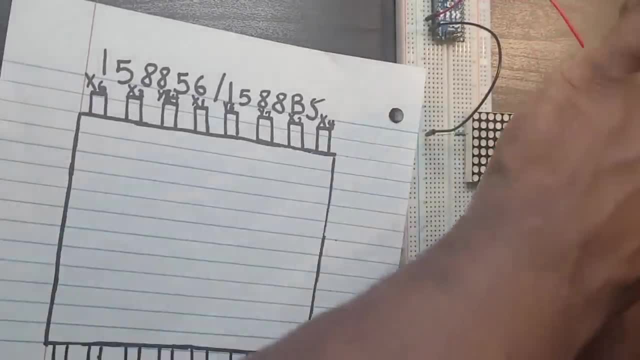 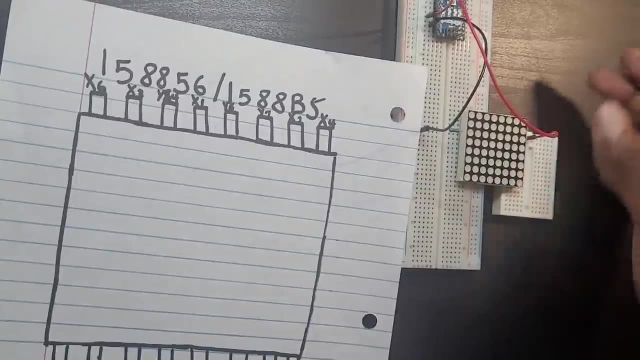 the five volt should be at x6, so should be at the one, and i'm going to put the five volt back to its place. now i'm going to push thezębemMedicOY over to the gnd. ok, and right now let's go back to the pson. at the very, very start, let me 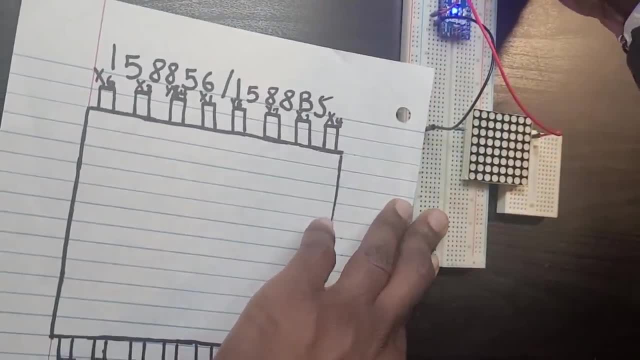 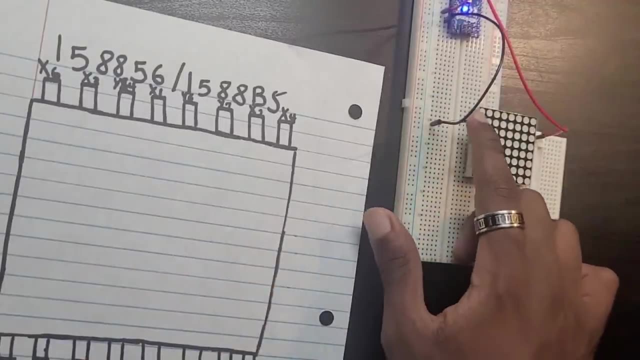 just there we go, the very start. let me just go here and i'll let me just plug in my arduino. all right, should be working. okay, it's not lighting up completely. let me just make sure the even the resistance is okay. there we go, the resistance of the problem. 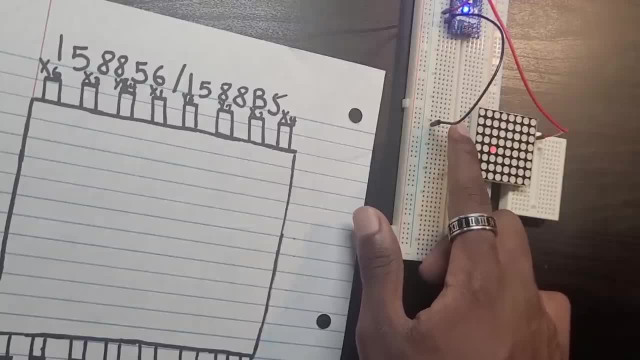 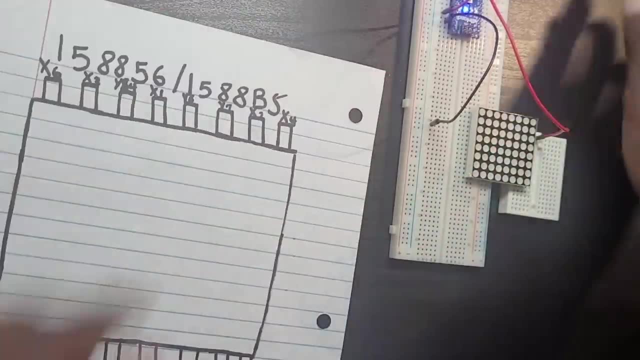 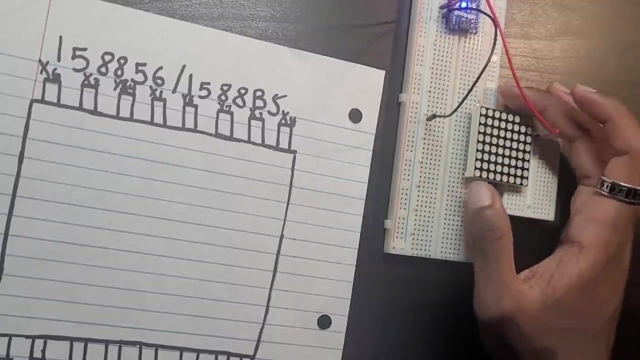 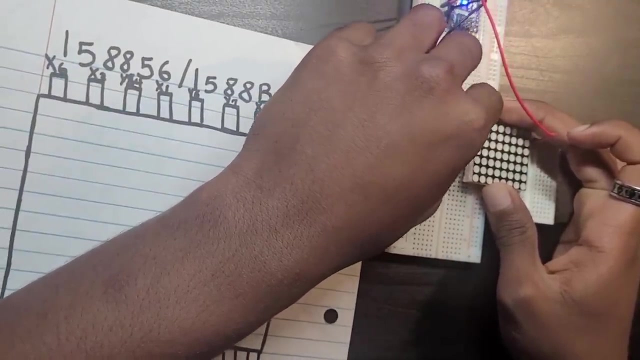 there we go. there is, this is the problem, but you can also wait. let me just the resistance. this keeps on. let me just take it off. I guess it's not doing well, let me get another resistor. let me get another resistor right here. it is really hard to actually connect these pins and see at the same time it's. 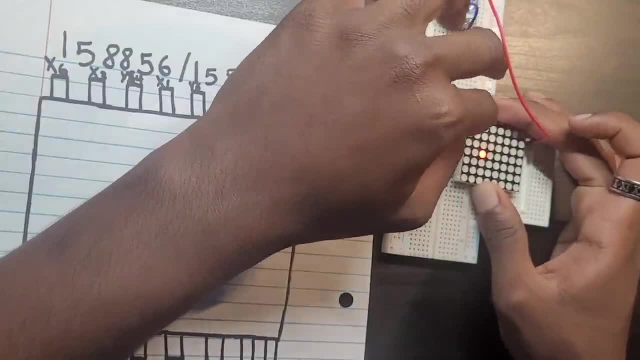 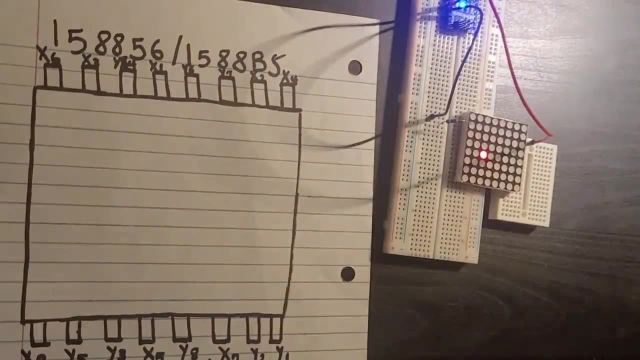 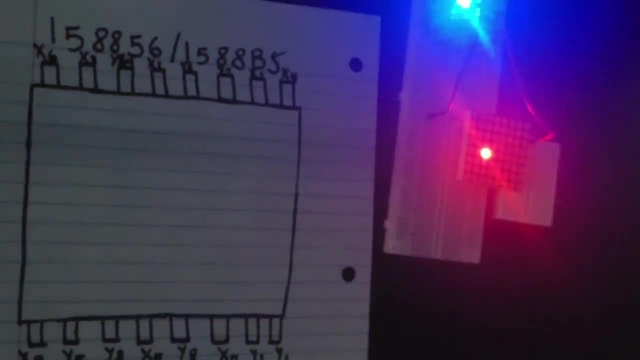 really hard. there we go. now it's even lighting up really really good. I don't think you might see it. it's lighting up even way brighter than it used to. can you see that? it's lighting up really really good. the last time I tried to light it up, what happened when I connect the 5 volt? when I connected? oh, let me. 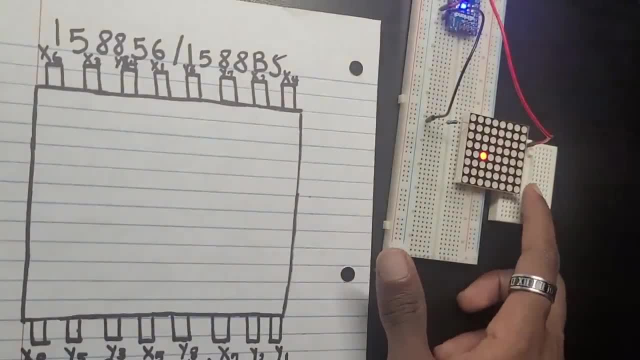 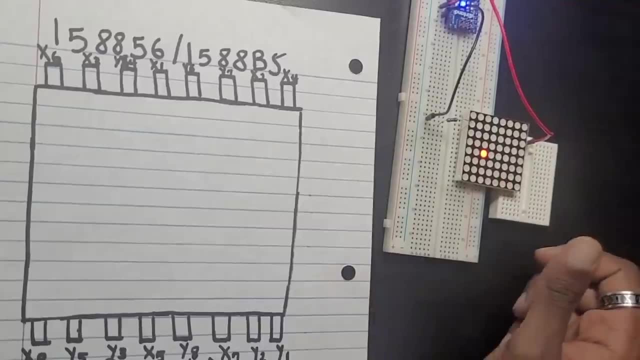 turn on the light so you can see it better. when I connected the 5 volt to the resistor, it wasn't lighting up that good. I can even see it myself. it was not lighting up that good. the problem isn't with the one thing. I want you guys. 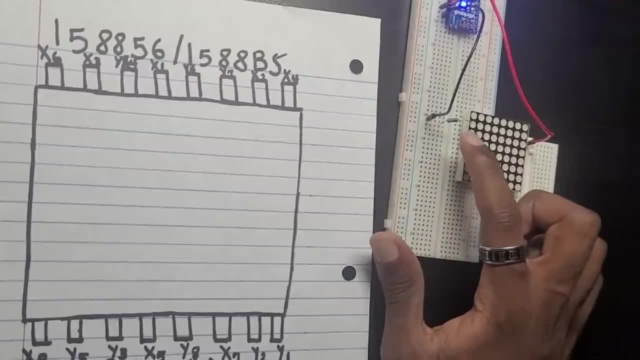 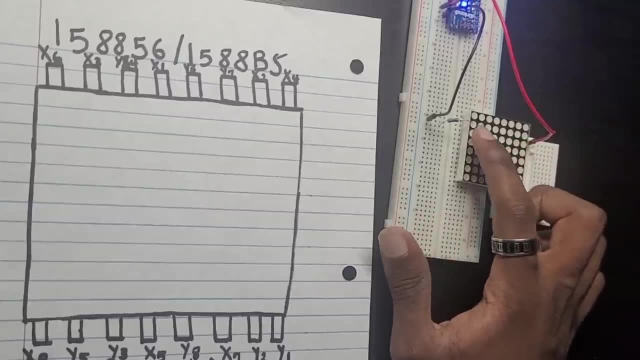 to keep in mind? is it's way preferable to do what it's way preferable when it comes to LED matrices? it's preferable to do what to go to what? to use our 5 volt directly and then limit the resistance? when it comes to the what to the ground, 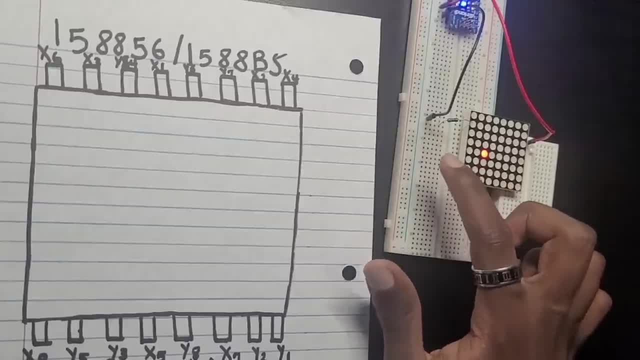 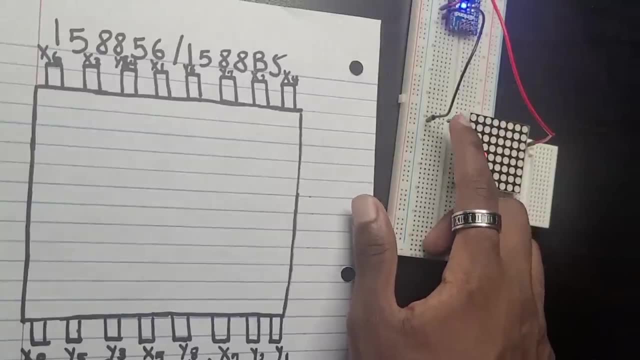 pin basically to the what, basically to the what, to the column. okay, that's one thing I want you guys to just keep in mind. so again, you can again wire it up as you like. you can wire it up again, put it to the what you can connect it to. 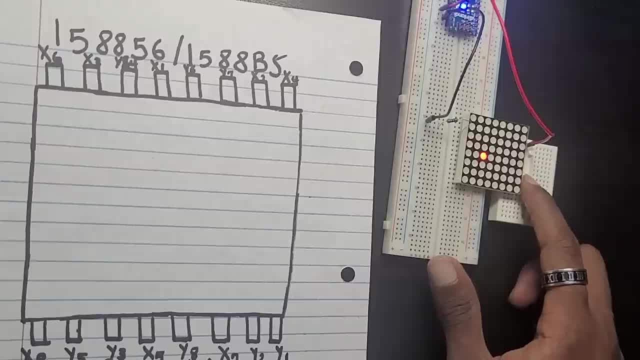 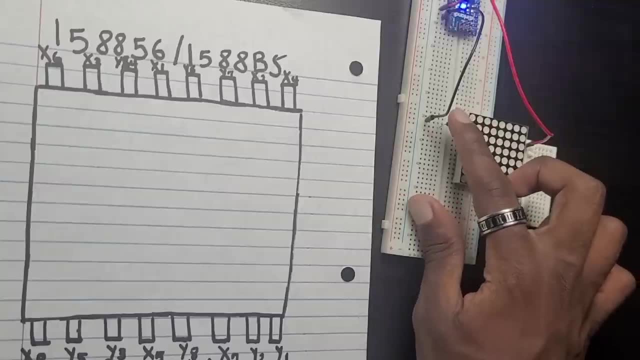 connect it to the pin and connect it to the resistor and connect it to the, the resistor to the what to the five volt. but it's again recommended that you connect it to the what, you connect it to, uh, the gnd. okay, because it's going to have what it's going to have more. 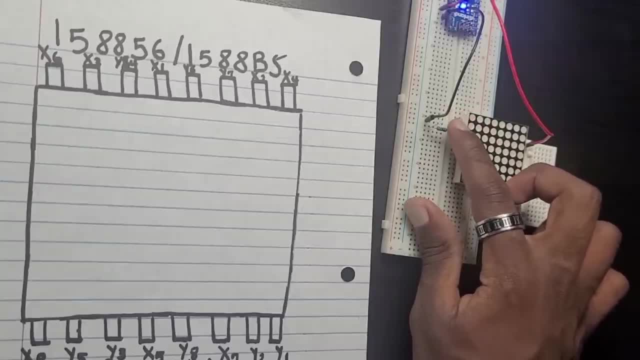 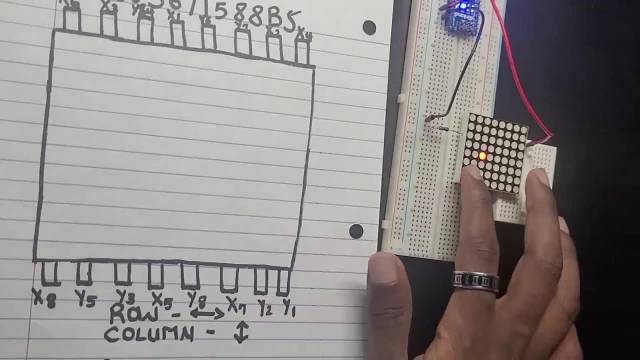 consistent lighting and it's going to be more brighter, especially when you're lighting up lots of led matrices at once. anyways, this is it for the section where we're actually going to be again checking what led matrices are and just introducing it, but we're going to work on a final 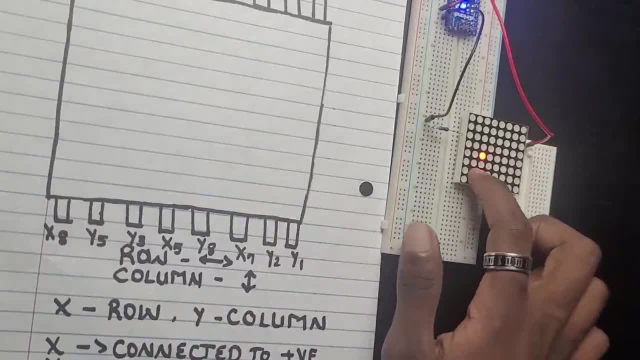 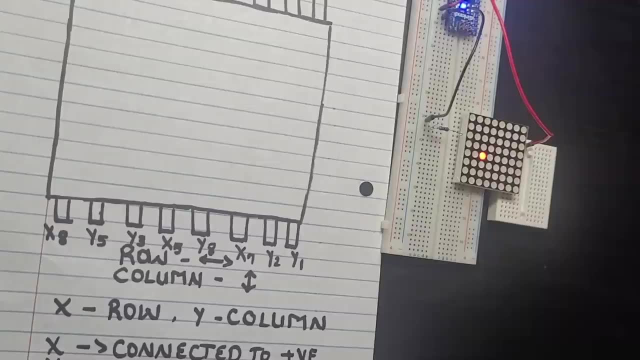 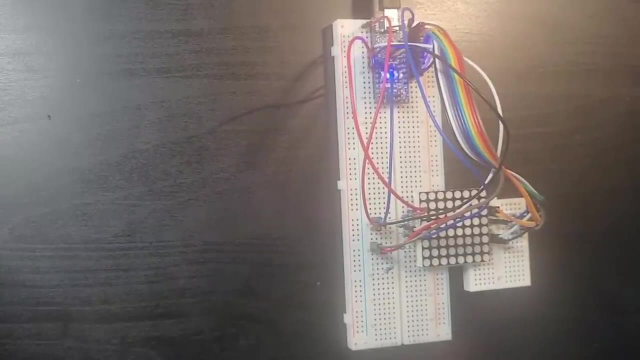 project before again, uh, before again, uh, moving on from our led matrices. so, uh, see you in the next section. we're actually going to work on a project involving led matrices. okay, so i read i wired up the led matrix, as you can see here. so let me just try to explain, um, what i did right here. so i just 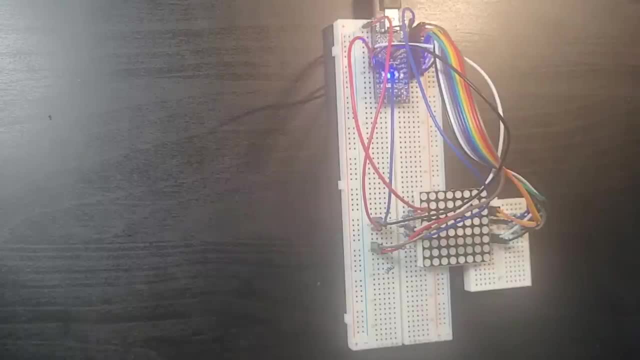 again write it up earlier because it takes a lot of time to wire it up, because there's like eight pins from the top and eight pins from the bottom, so total of 16 pins. so it's going to be a really, really it's going to be a big effort to do what to actually. 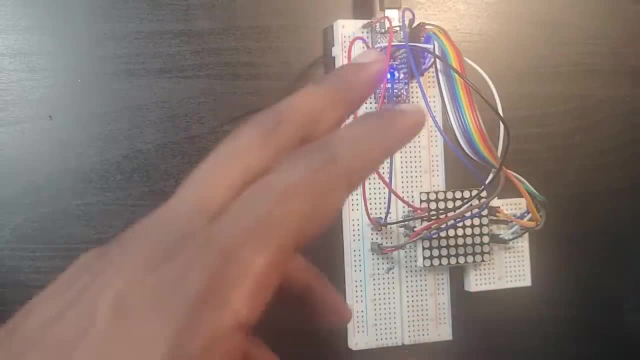 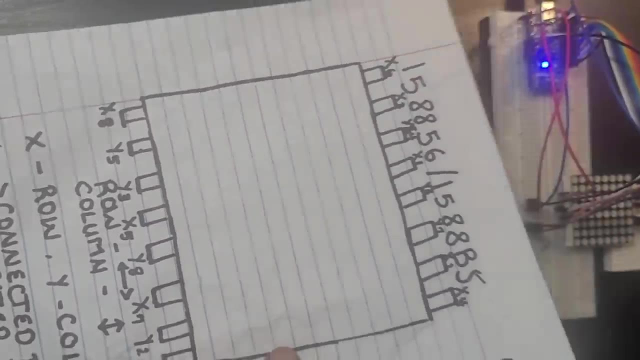 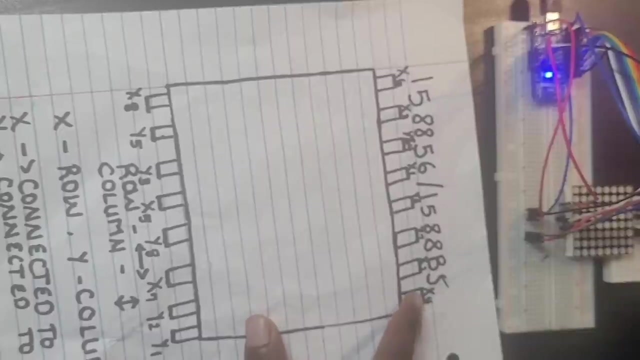 connect the what, connect the led matrix again to our arduino. okay, so right here again, this is my um. let me just bring this bit back so you can see it. this is basically my what. this is basically my documentation on what the documentation i made on my uh, on my led matrix. okay, so right here is what. 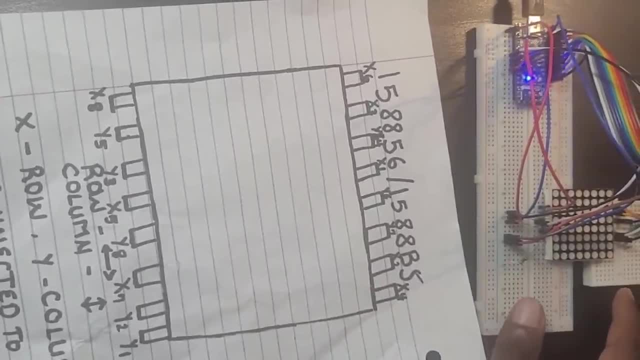 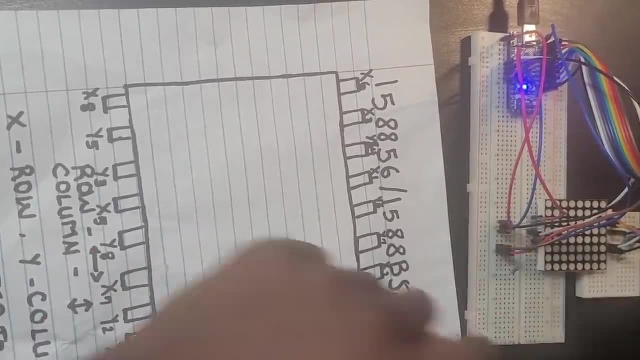 this is row four, connected to the black one. let me just go right here so you can see it connected to the black one and then the white one. i keep connecting this again with the parallel wires that are here. okay, i'm just going to be connecting it. the wires that are next to each. 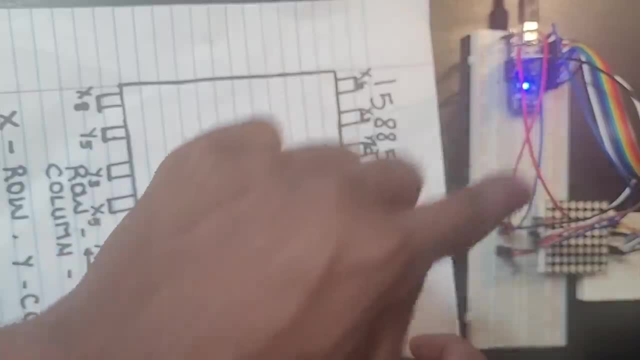 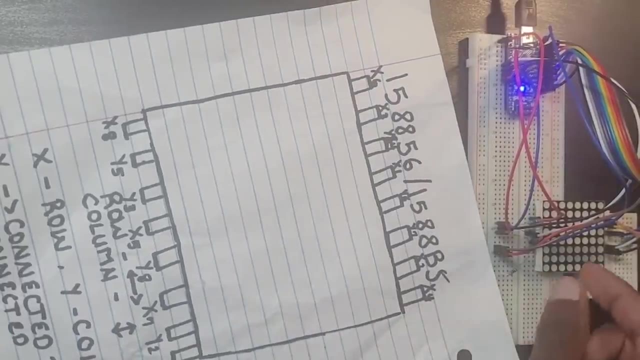 other. so i keep connecting it all the way up to here and then connect it starting from what? digital pin, uh two. okay, so i keep doing that and then, once i'm done with that, there's going to be two pins left here, these two pins right here, these two uh wires left here. and i start from here and again. 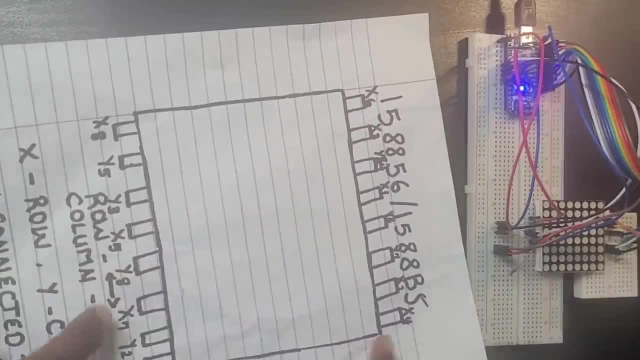 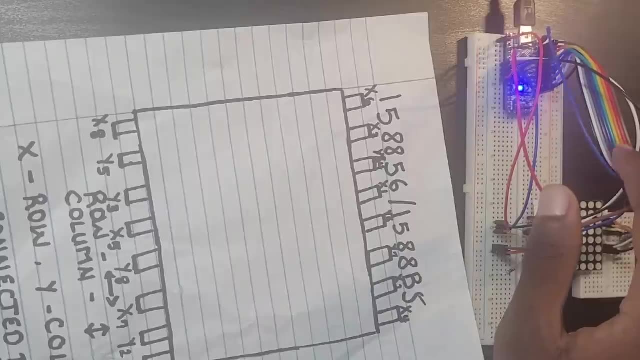 what do i do? i keep going on again, i keep going on. obviously, the wire ends at a 10. i connected eight here, then i connected two. there's a total of 10 wires here. okay, so what happens is what? i start using the normal wires, as i said again, so i run out of it. 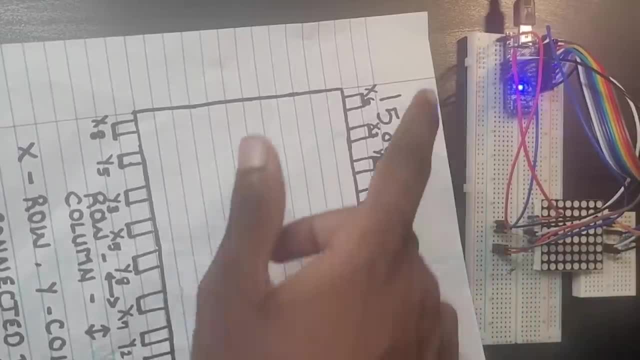 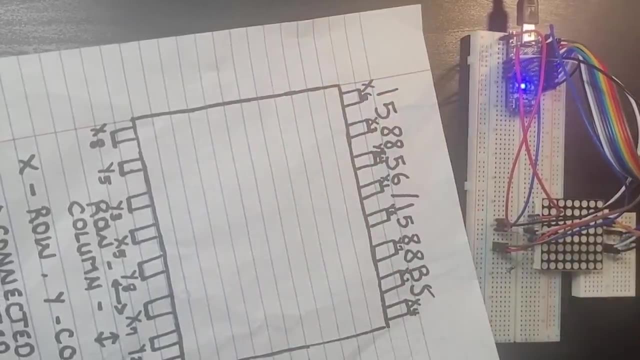 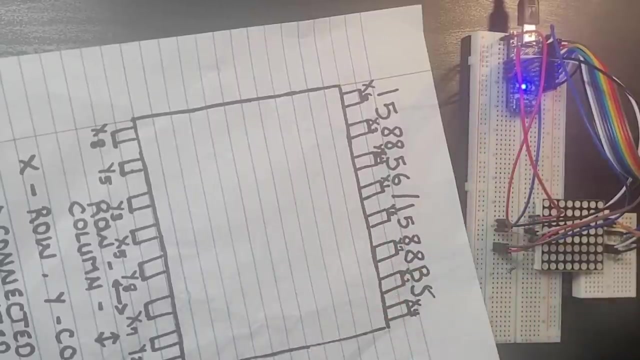 so i use my normal wires and keep what and keep adding it up until digital pin 13. after digital pin 13, we run into a problem. what is that problem? we have 16 pins here. okay, we have 16 pins. and right here. how many pins do we have right here in the arduino? additional pins we have around? 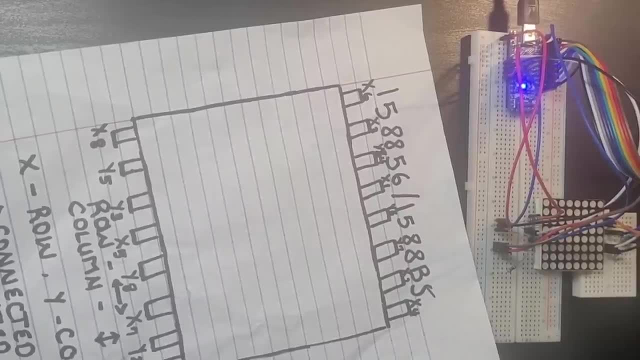 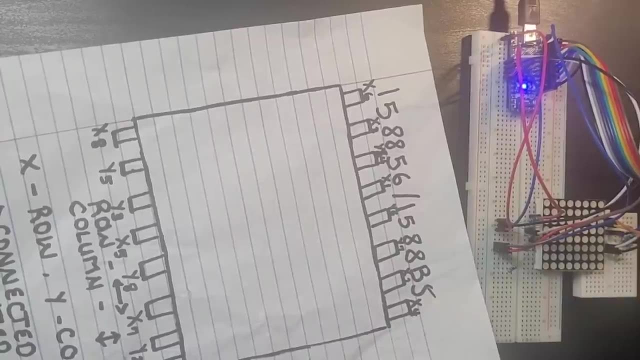 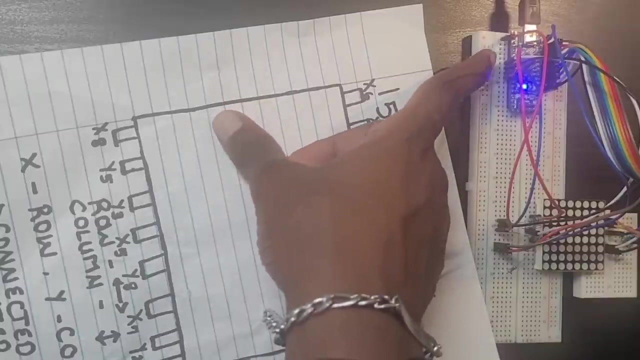 how much maximum of what maximum of 13? in my arduino nano, specifically in my arduino nano, there's a specifically what there's specifically the maximum is what? 13? what digital pins? okay, so we run into this problem. so what do i do? i try to use the analog pins afterwards, so i start to 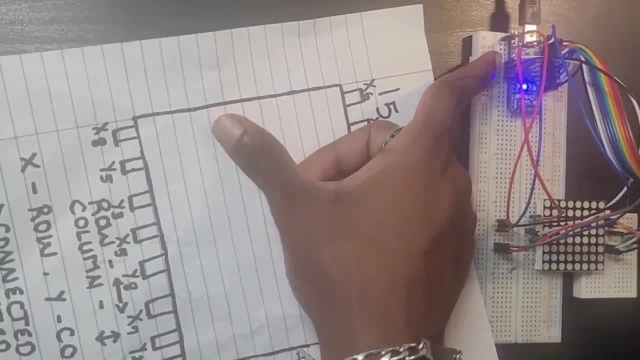 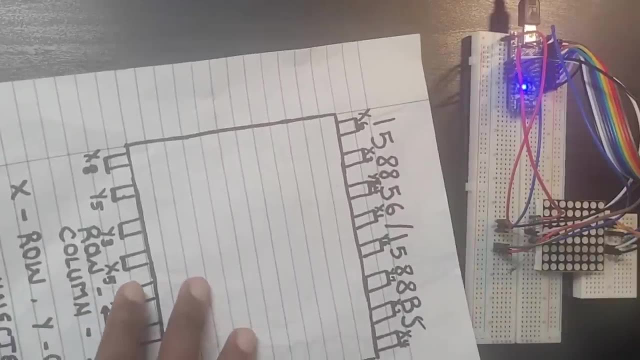 use the analog pins. i think starting from a2, let me check. yeah, starting from a2, i start to use the analog pins. okay, connected them again. it's going to be what different again how you wire it up again. what is the number of pins? again, i can go one by one, or maybe i can go per square root, or maybe i. 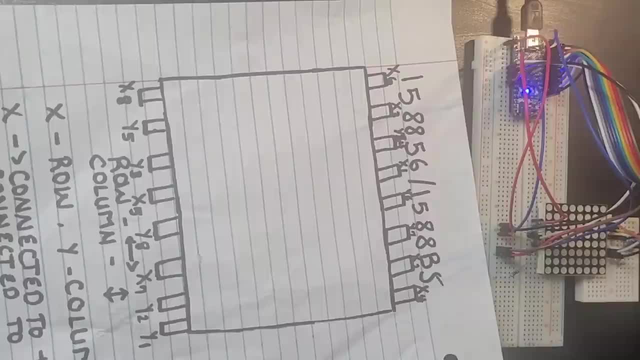 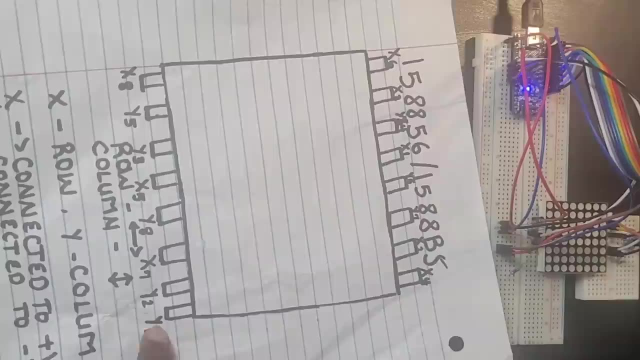 can do it by one-and-a-half by one-and-a-half by one-and-a-half, but it's going to be different depending on what kind of pin that i use. you're going to have some of these. these are not going to be the same because they're going to be different from person to person, depending on the. 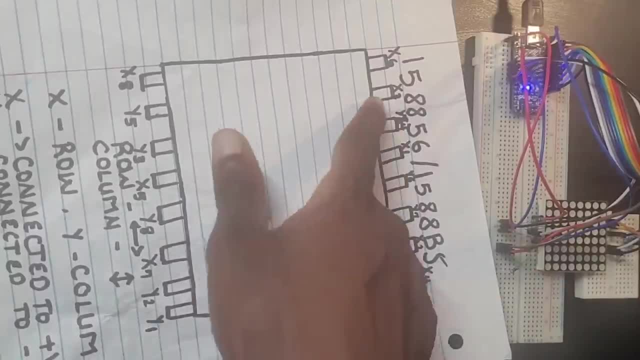 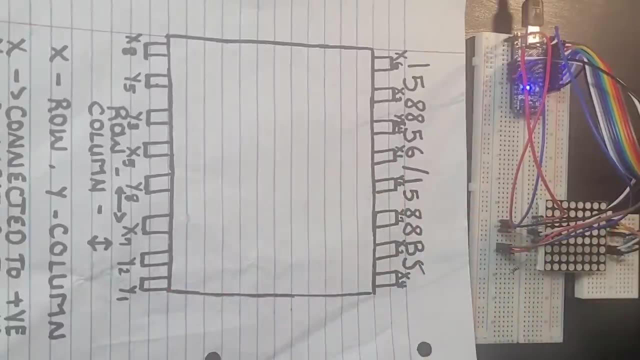 model of what the model of led metrics you have. obviously they'll look the same, but obviously the number again is going to what it's going to affect where, um, every other pin is going to be. so every column right here is going to be what my column one is going to be, here, right here, at the very edge. 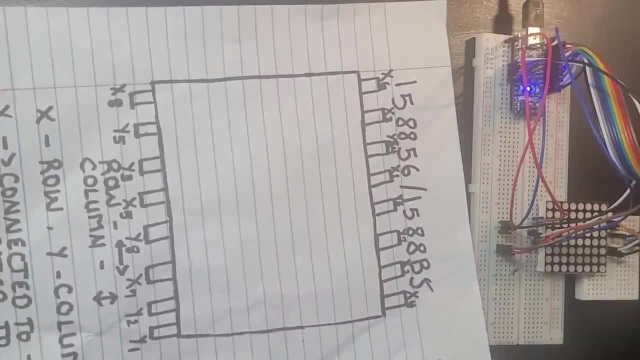 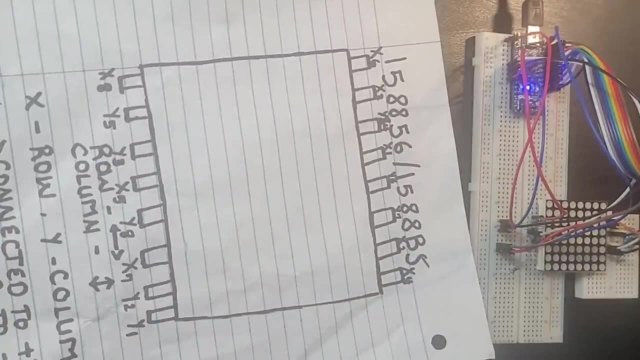 of the led matrix. okay, so i just want you to keep this in mind. so again, this i made is again specifically for me. how would we know that? i already showed you, guys. what you need to do is keep on wiring it up until one lights up. as soon as one lights up, what happens as soon as one lights? 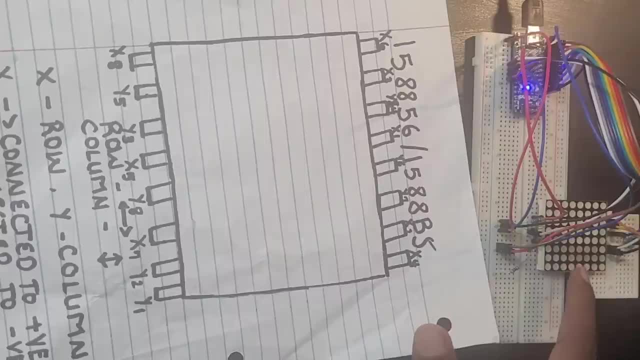 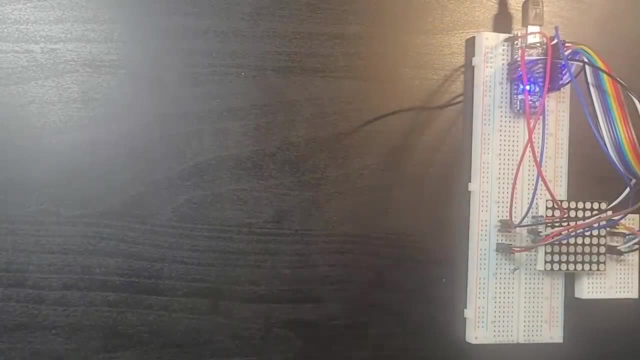 up. we can extract two information from it. we can extract the row and the column. okay, okay. so, with that in mind, okay, let me go over to my code. and to even check that everything is wired up properly, what do we do? we're going to need to turn on every led matrix right here. we're going to need 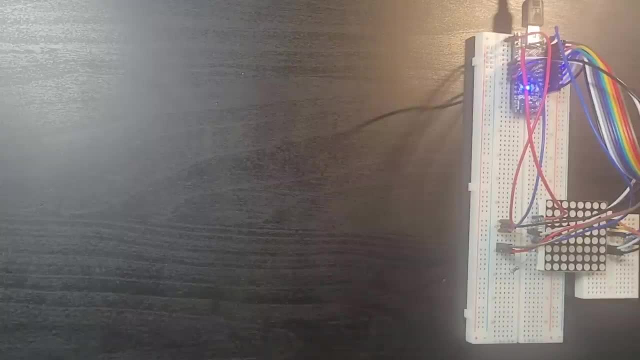 to turn on every column and every row just to see that everything is wired up. sometimes, again, what happens is what the resistors? again, they might be attached together, sometimes they're not put in properly and sometimes we run into what physical errors, so sometimes it might confuse us. 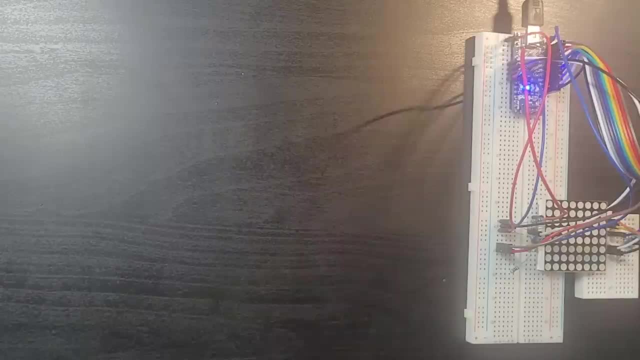 where the error is occurring. so your code might run perfectly, and then again you might have a problem when you're working with the led matrix. it happened to me when i was working with the uh, for what? 14, 14, 7 segment led display. okay, so with that in mind, how do i turn on everything? so let me first again. 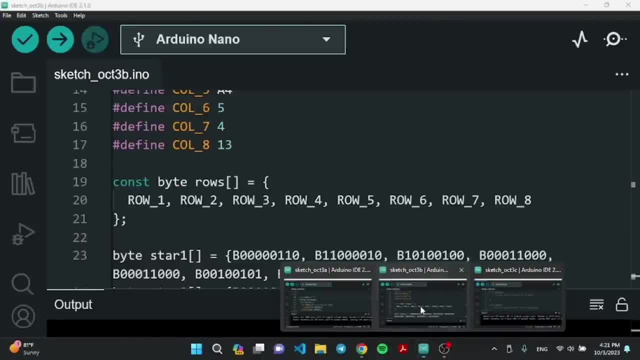 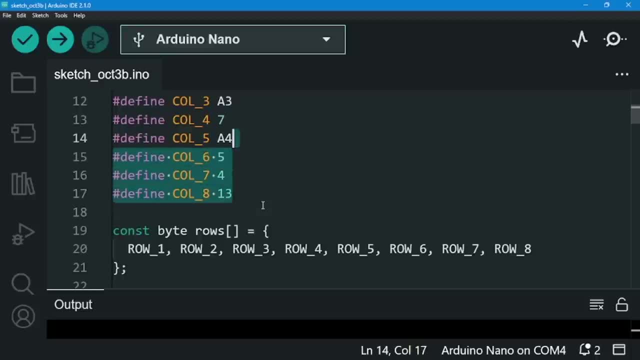 there's. i defined them earlier right here, so i don't waste your time trying to do that. so i define them right here. basically, when you use the keyword hashtag define, it's basically like using variables instead of here. they're going to be what, they're going to be set to constants. variables are what. 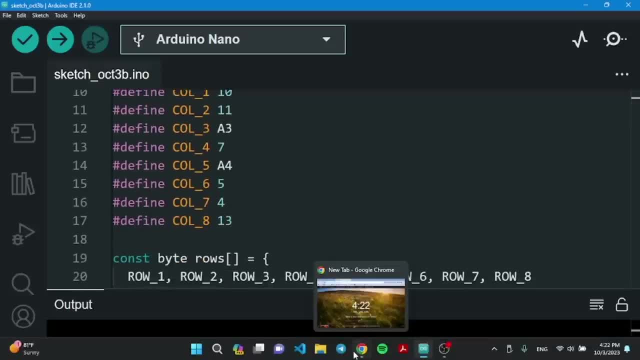 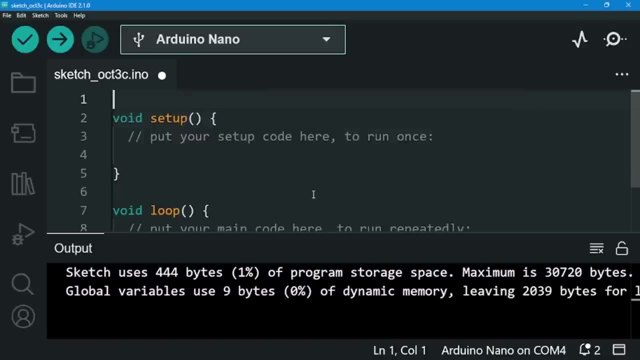 they change from time to time. again, you can add them up, you can what, you can change them, but when it comes to what? when it comes to constants, they're always constant. i just want to think. let's say the constant of gravity is what we're going to say hash to define. okay, i'm going to say hash to define for uh. 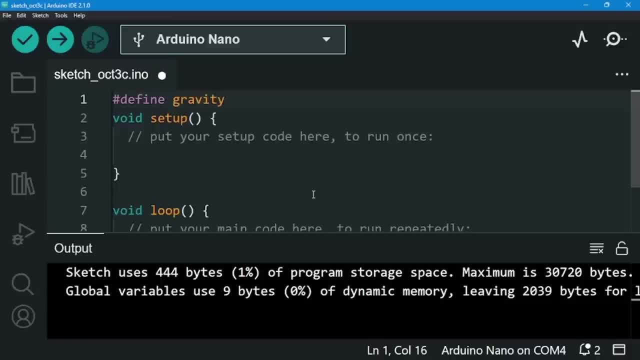 work anywhere. after defining, we're going to be saying gravity. gravity is a constant. what is it? it's 9.8, 9.8 meters per second. so we're going to be defining constants. okay, so it's exactly going to do the same thing. as what? the same thing as variables, but it's going to be what it's going. 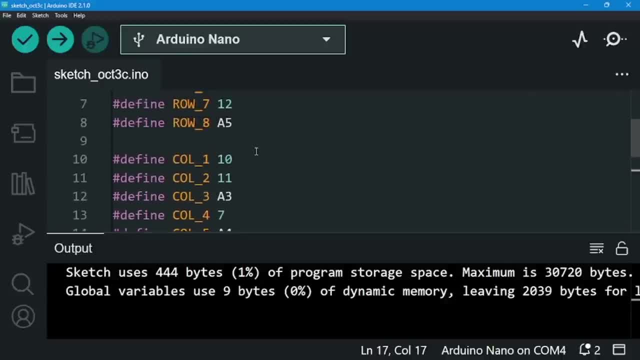 to be set to constant. it's not going to do it. you cannot change the value once you set it. okay. so i'm gonna set it up to what the actual value $3 gets by using this. so what value does this value that we're going to say it? 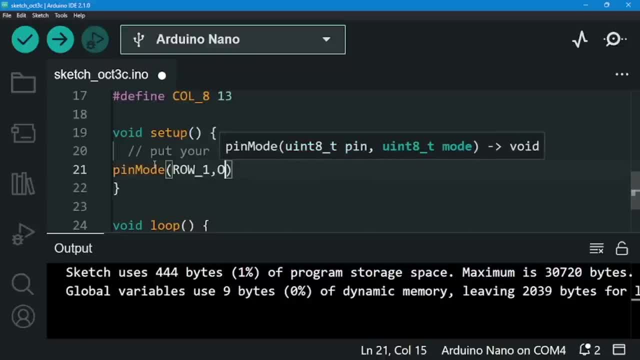 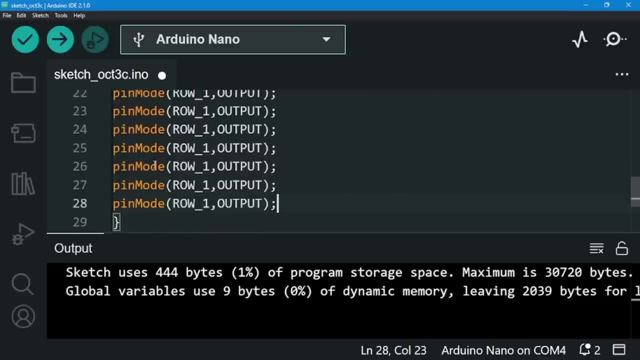 get applied to driven by what it will do, even bigger, okay, and then i can workflows here. so let me go to bronco, monetize these two. i'm going to point back and i'm going to use my form to define the values of the next time that we will microsoft. what i'm going to do is we're going to define. 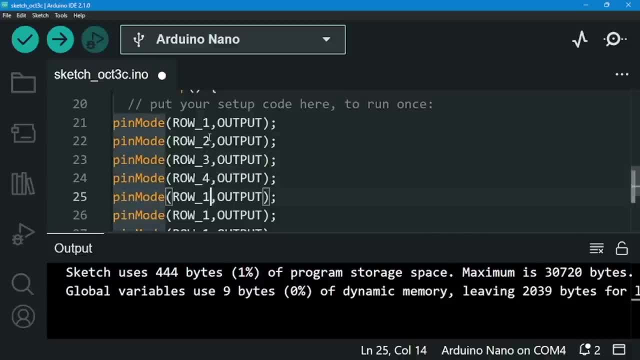 them up to eight, right? so i just set this up again. i define the row one up to eight and what again? pin, again, pin they're connected to, and then column to what? column? one to eight i just put. i just roll them down to row two and then row three, row four, row five, row six, seven and then finally eight. i'm going. 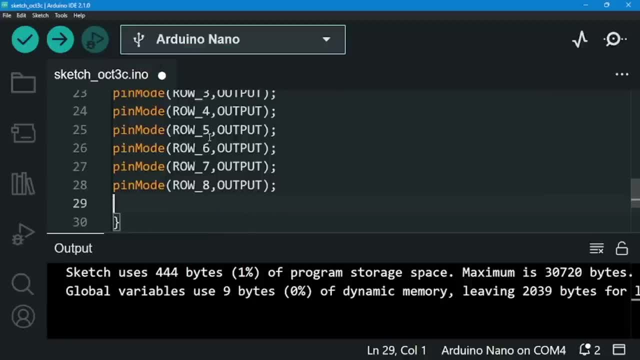 to be doing the same thing when it comes towards what. when it comes towards- oh wait, i'm not correct here- when it comes the same to the what to. when it comes to the columns, too. let me set all of them to what to output. that's what i want to do. i'm going to be using all of them as an output, okay? 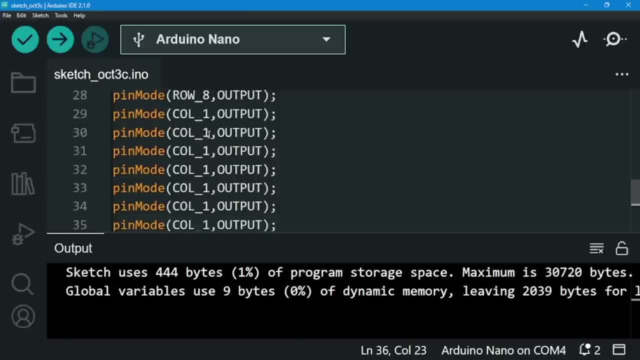 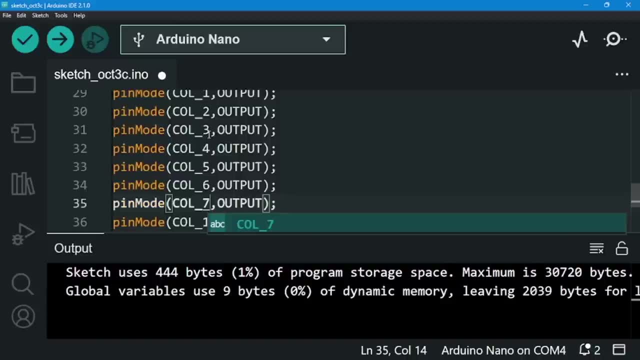 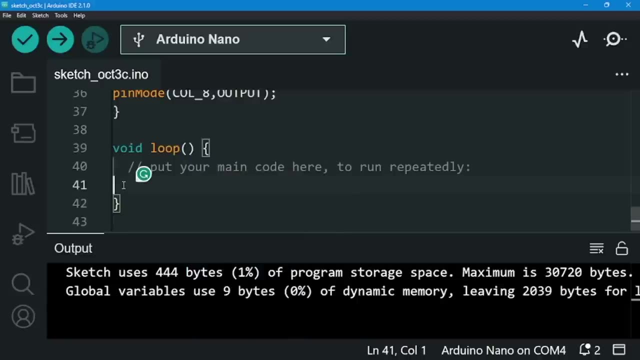 so let me paste this again. go pasting it, and i think this should be eight. we go two right here, three, four, five, six, seven and then eight. there we go now afterwards. what do i want to do? turn all of them on. as you remember, we're going to be setting what the rows to high. 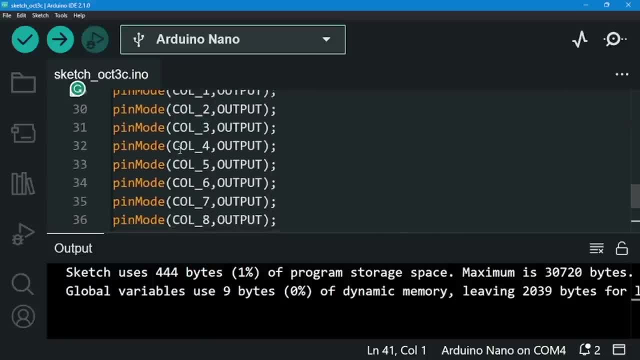 and the columns to low. to light up what? to light up even a segment of the led matrix, if you remember. so, to even light up everything, i need to set all of the columns to high and the columns to low. to light up what? to light up even a segment. 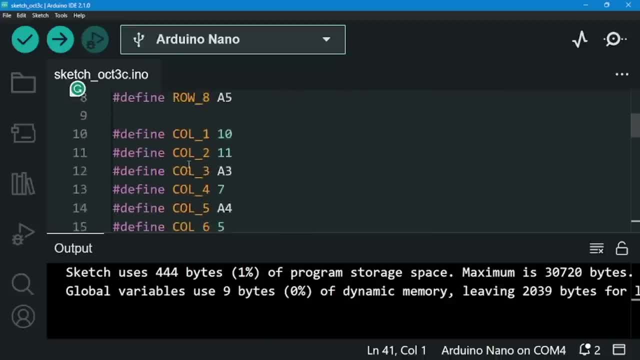 all rows to high. but one thing i want you guys to again pay attention here is we used analog pins and also what we also used digital pins. so, depending on the pin that i have, i'm supposed to say, i'm supposed to be saying what a analog right for analog pins and for those who have. 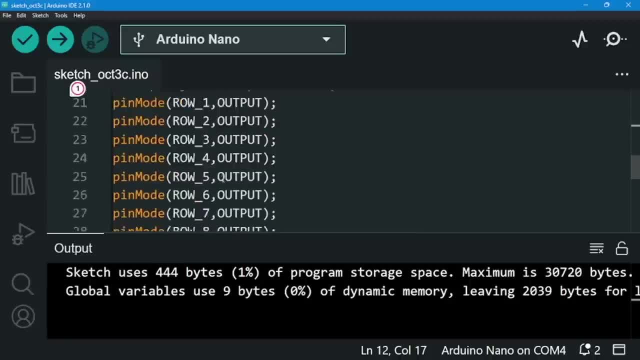 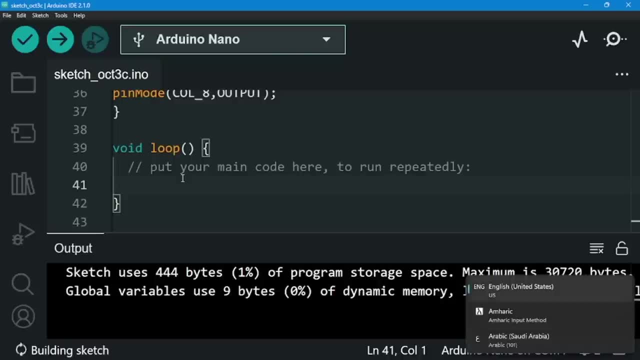 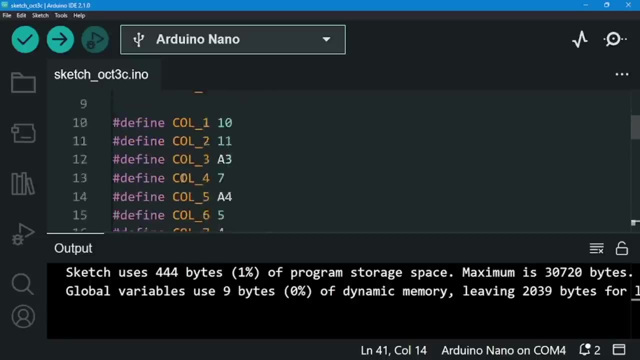 again: additional pin. i'm going to be saying what? digital right, okay, so i just want you to keep that in mind. so let me just say: there's the right right here. oh, exchange my language, let me just. there we go. well, let me just turn this caps lock off. there we go, digital right. then let's just check which rows receive additional. 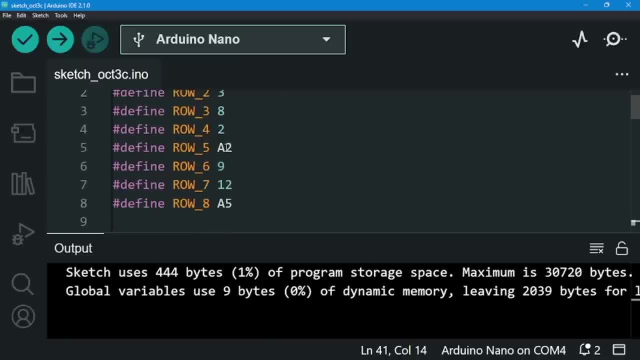 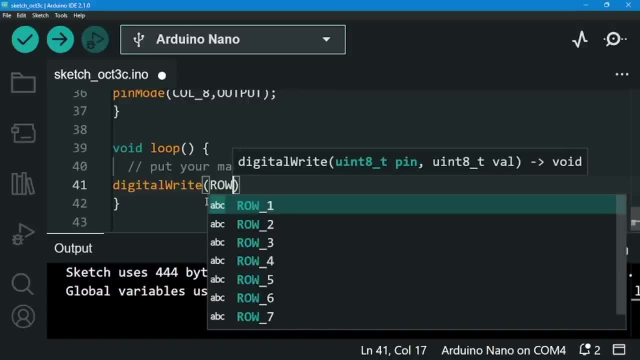 right. so all of them seems to be receiving digital right, except for row five and row eight. so, except for rule five and row eight- i'm going to be saying this to right. i'm going to be starting from row one, row one and setting this to high. 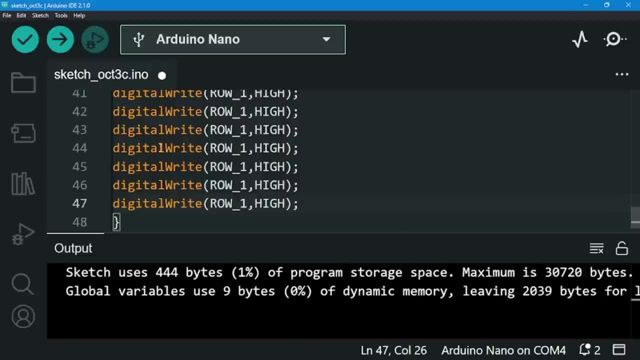 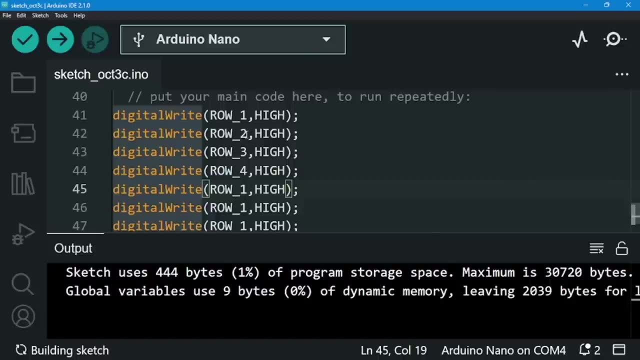 and let's keep just pasting it a bit. there we go, and now for row one, we're going to say row two, three, four, we're going to skip five. we're going to be using analog right for five, five. then we're going to go six, seven, we're not going to be even writing down what- eight. 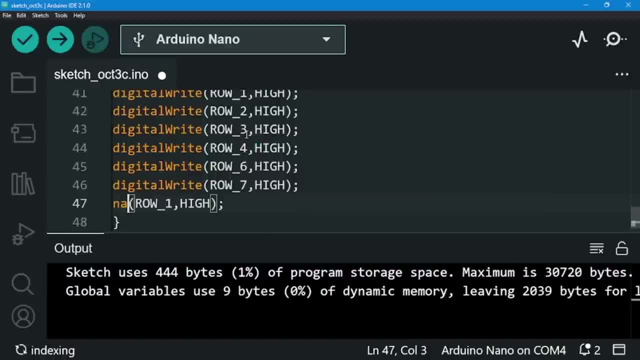 eight is going to be using analog right. so let me go here and say analog right and then if i set this, let's say set it to row five right here, and then i cannot use high. when i use analog right, i'm supposed to be writing down a value which is going to be an integer. 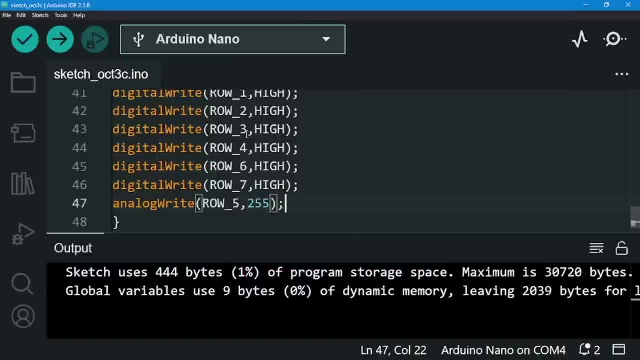 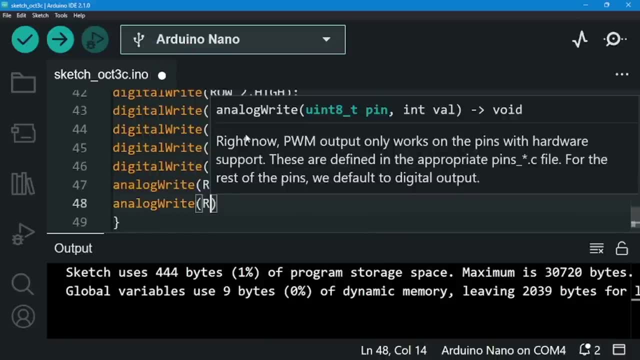 between zero and 255. obviously, high means what? 255? so i'm just going to be setting it to 255 right now, and then, once i'm done doing that, what do i do? i'm going to be also copying the same thing for row eight. row eight: set that to high, obviously, right now. oh, i'm supposed to say 255. i said high. 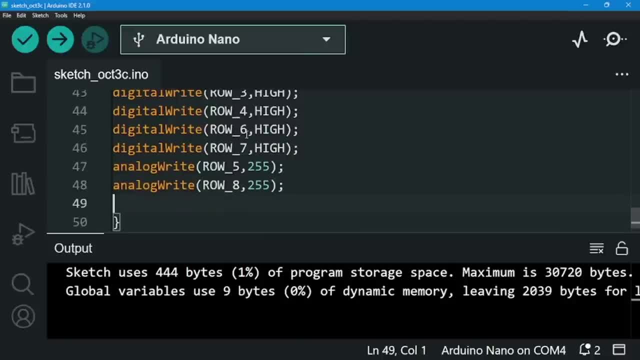 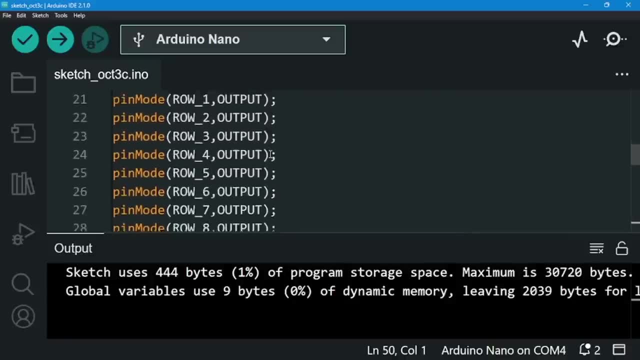 instead of 255. my bad um. so after this, obviously our job is not done. now we should set what the columns to what. we should be setting them to low, or basically gnd. okay, so column: uh, most of them are going to be set to low, and then i'm going to be setting them to high and then i'm. 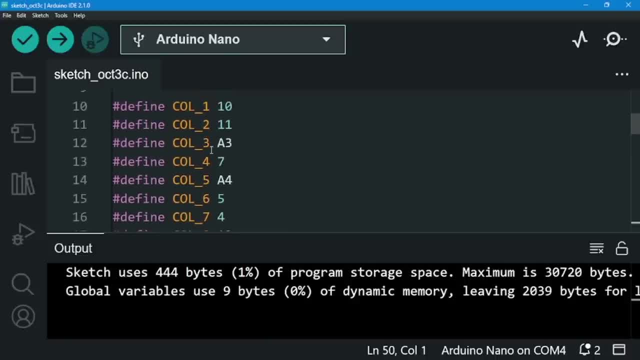 going to be setting them to low, and then i'm going to be setting them to high, and then i'm going to using it. yeah, only two of them don't use it, and this time they're what? column three and column five. okay, so okay for columns, what am i going to say? they're still right. most of them are going to. 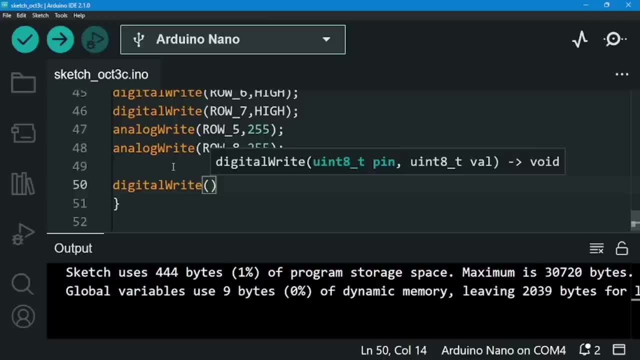 be using digital pins again. it's because i run out of them that we're going to be using analog rights. so if you, if you guys, have an analog pin- that again your arduino, again your type of model that has more than 16 pins- i suggest that you use only digital pins. okay, mine does not have it. so 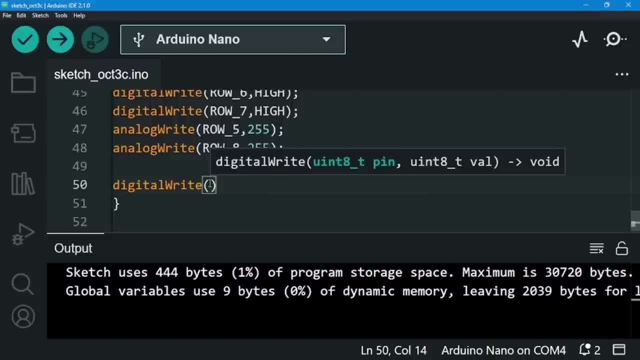 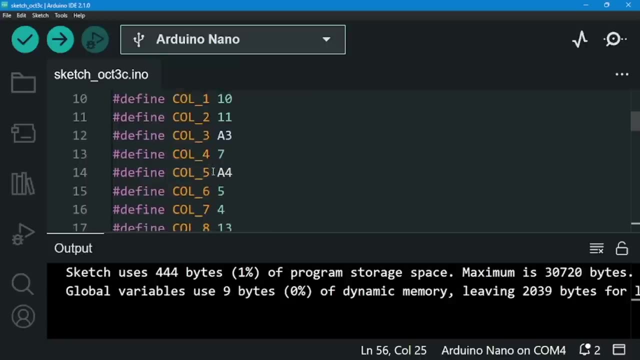 i'm going to be using analog pins too, because mine is a bit small, okay, so let me just say: column one: two, low. we set that to low. let me focus on the numbers here. one number, okay, there we go. column one: two: okay. column three and five are not going to be what they're going to be, using analog. 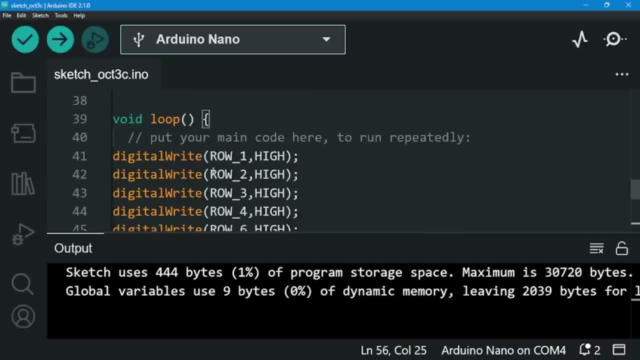 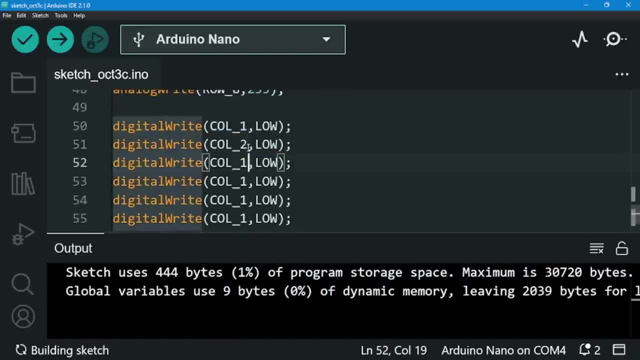 uh, analog, right. so except for them, three and five, i'm going to be using everything. so let me go to column right now. let me go column two, three is not going to be using it, so i'm going to be skipping three and going to four and also five. we're not going to be what, we're going to be using analog. 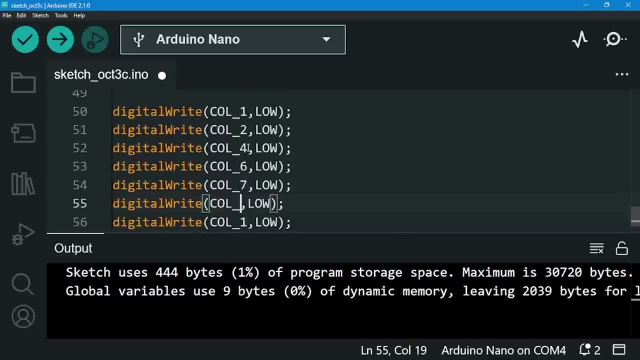 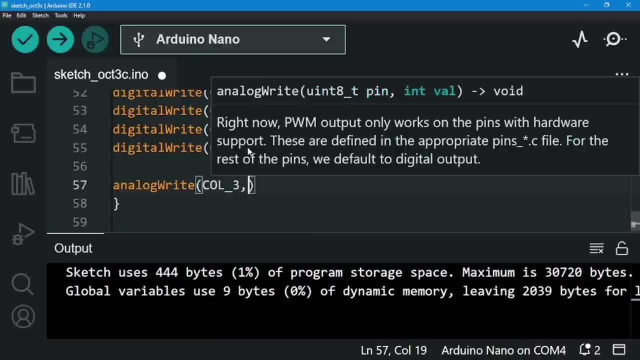 analog right, and then seven and then eight. let me just remove this code. all right, there we go. now I'm gonna be writing down panel log. let me turn off caps lock and lock right column. we're gonna be starting from column three and then setting it to what to zero. zero corresponds with what with low. all right, 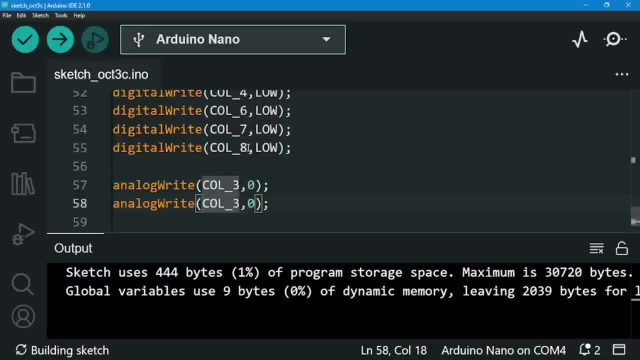 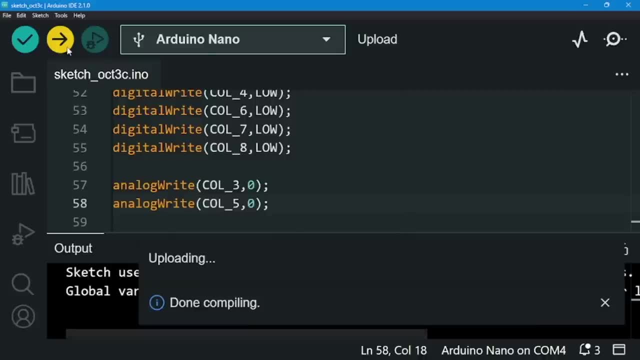 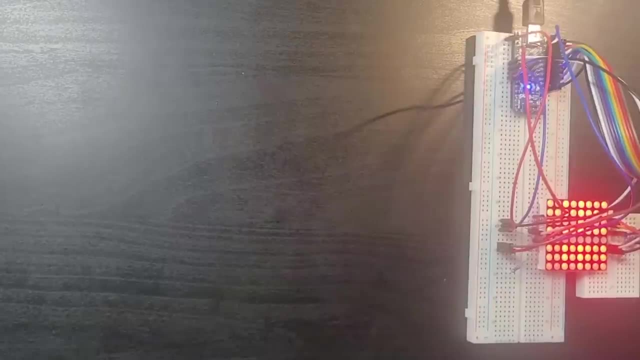 and then copy this and then do the same thing. for what column five? there we go, and now I think everything should light up. let's just upload the code right now. it's done compiling and it should be done uploading. can you see it? almost everything is lighting up. let me just turn off the light for you guys, so you. 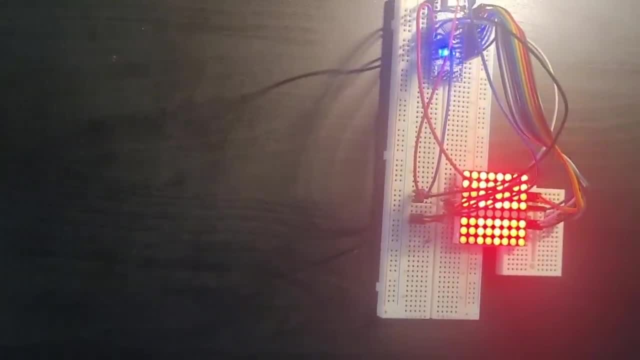 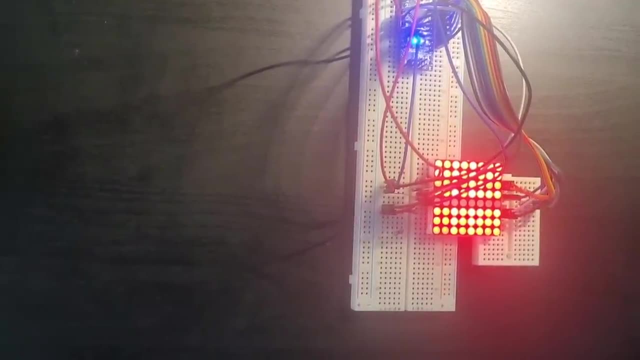 can even see it better and change the angle here- it's not the best of angles. there we go and just move it a bit. there we go. you can see that, uh roll, what a column. what column one, two, three, column five is not lighting up. so basically I 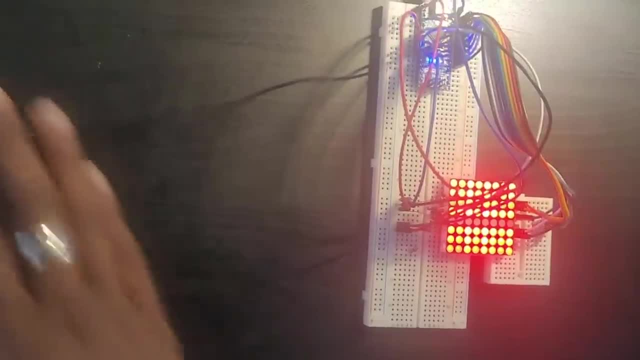 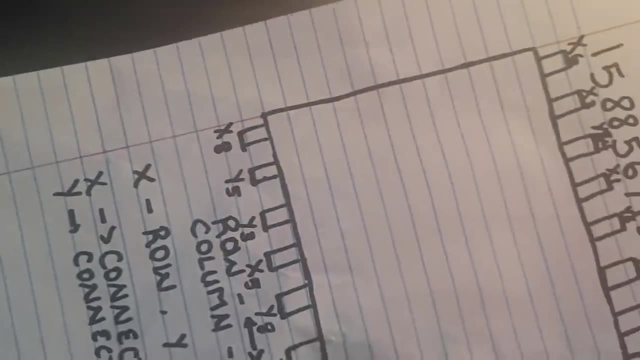 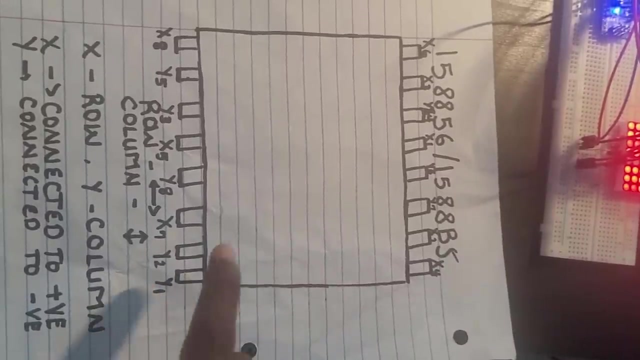 have to touch the resistor or something. most of the cases, again, resistors, uh, they're not put in properly, so let me just check my documentation right here to understand which one is causing me some problem right here, okay, so column column five should be around. should it be around, it's not here. okay, it's here. 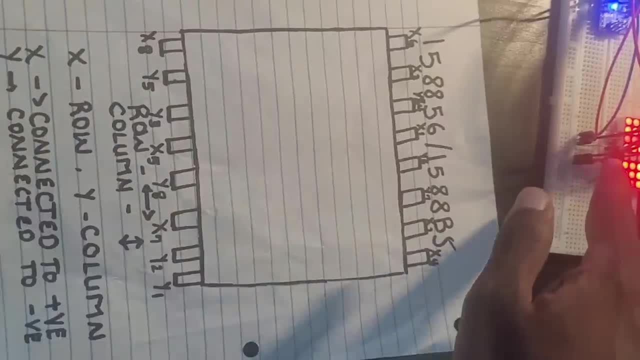 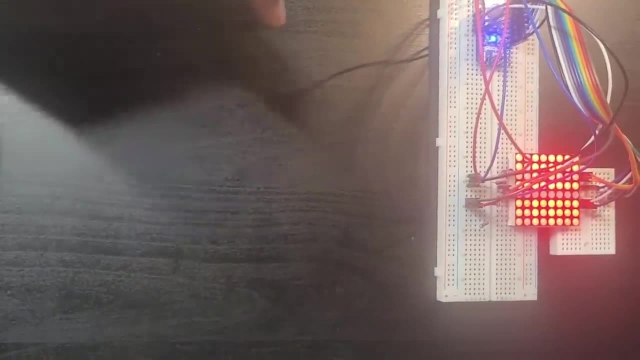 there we go. column five is here, so the resistor that is at the very front right here- let me just turn on the light so you can see it- there's a resistor at the very, very beginning. there we go, at the very, very beginning. I'm just turn that. 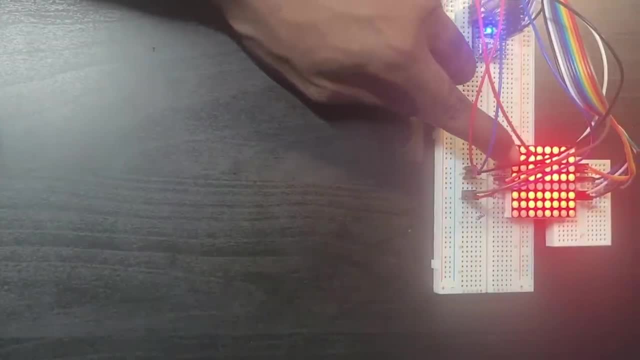 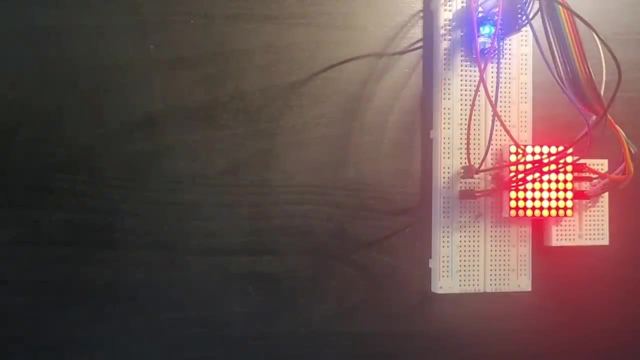 off. there we go, just touch it a bit, don't touch the other ones. there we go, just touch it a bit and turn off the light so you can see it better. now everything is lit up. there we go, everything is lit up. okay, so everything seems to be what? 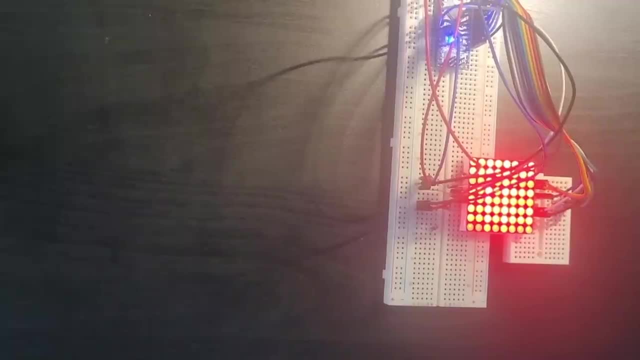 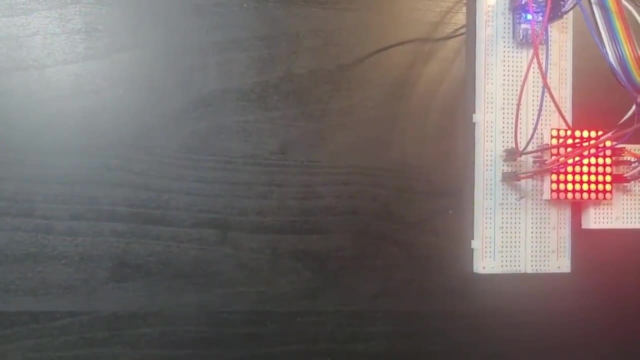 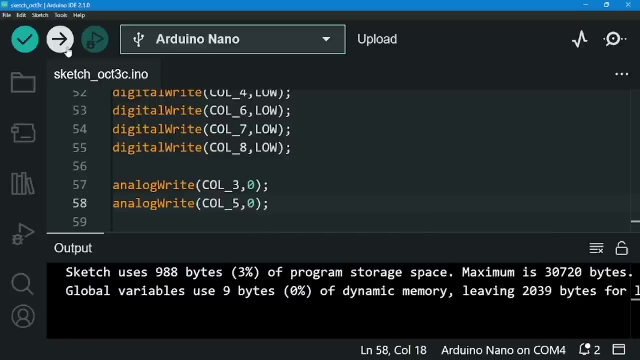 connected properly. so every column and every row was connected properly. okay, that's good. now let's try to again do something interesting with it. so obviously this tried to do what a project with. so right here, what we're gonna do is: okay, I'm gonna be having. I've tried to actually search. 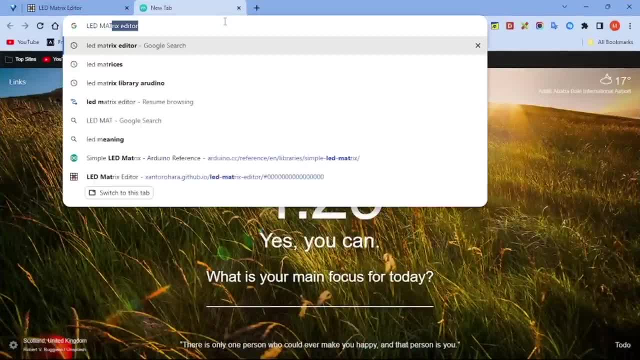 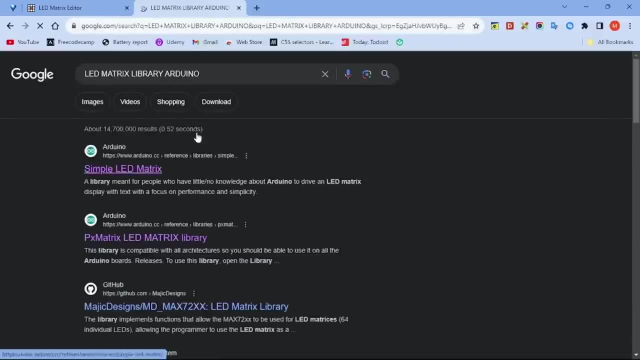 for libraries. okay, I've searched for LED matrix libraries, just like how we had the safe sec library for the segment LED displays, the seven segment LED displays. I try to find LED matrix libraries and when I did that, what I found was most of them requires something called a max 7 to XX chip. basically, it's not gonna be. 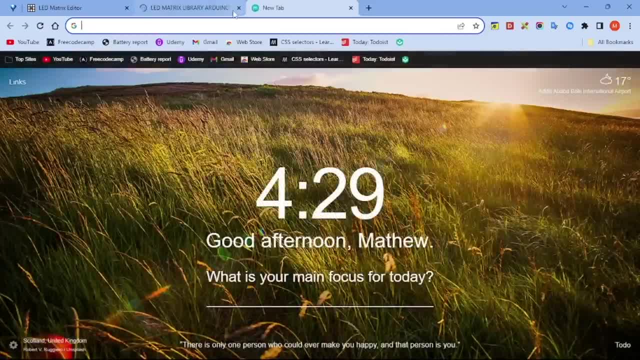 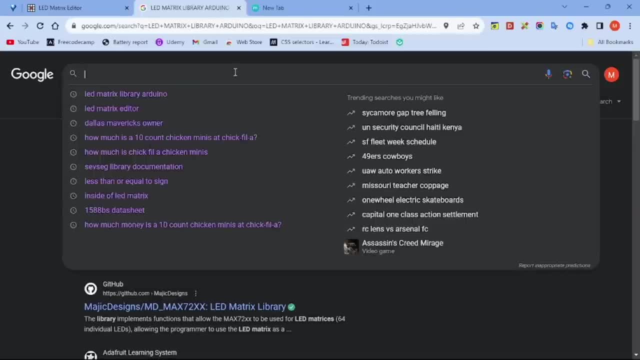 your typical what your typical LED matrix. it's gonna have some like some add up to it, all right, so it's not gonna be exactly the LED matrix that we're using right here. okay, so it was limited to what? to the again, the models that are what the? 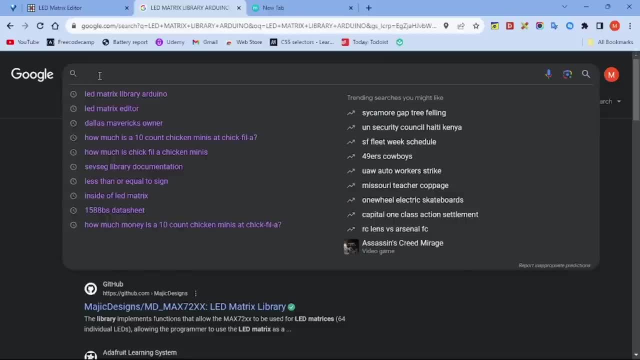 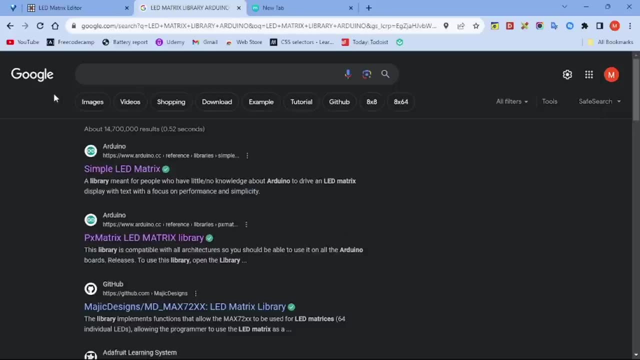 models that are popular. mine is a bit of a less known model. okay, not only that too, but it's gonna include its own chip. so it's not gonna what. it's not gonna include the traditional LED matrix. when I look at most of the what most of the 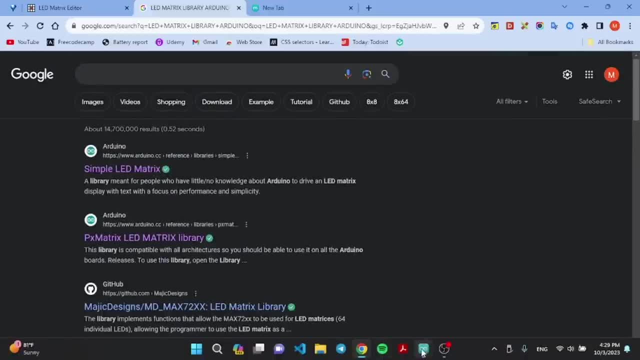 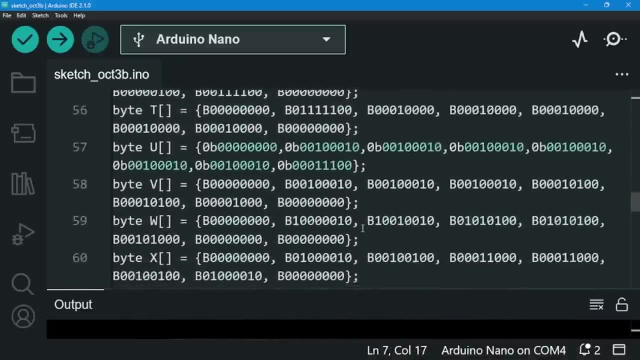 libraries. okay. so what I did was: let me just go over to a code right here and let me go over to the code right here. there's a code right here that is preset. okay, I don't want you to focus too much on this. uh, what all of this is. but 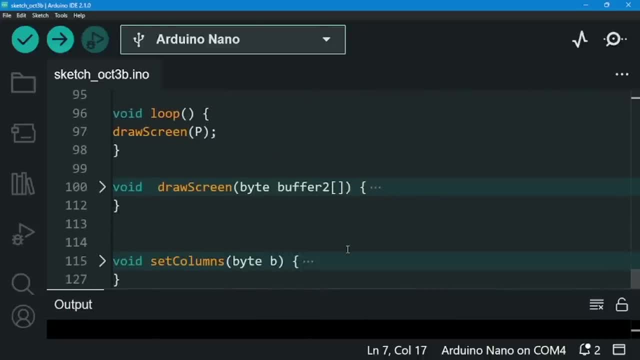 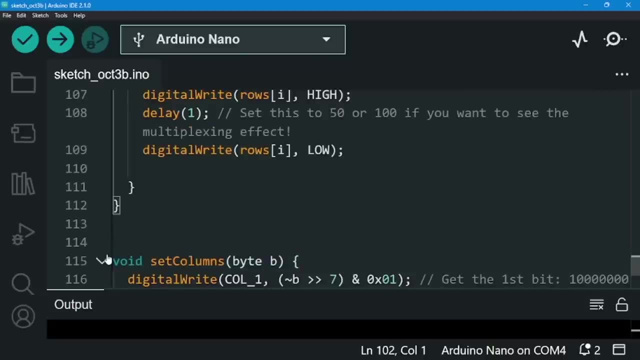 there's a preset code right here that I'm going to be leaving down in the link below, the link below in the description below. so again you guys can see it and you guys again can use it for yourself, so you can again get the sketch for yourself, okay. so let's just analyze the code, though we're not going to be just 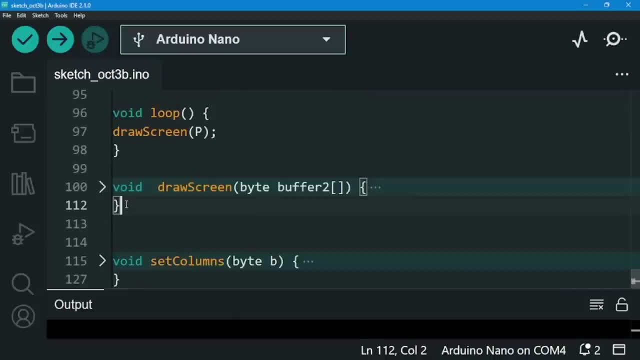 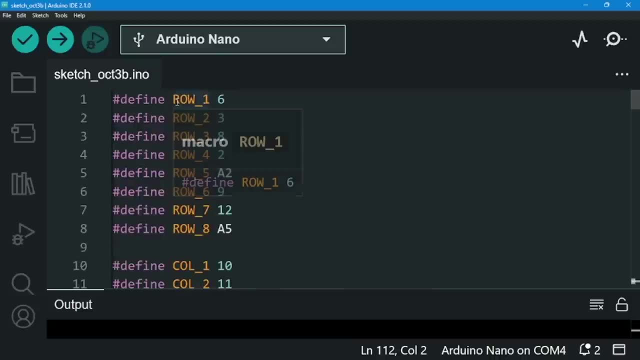 giving you. I'm not going to be just giving you the code, okay. I'm just going to let you analyze too, what you need to analyze, okay, so let me focus right here. so let's start with. it's going to be defining again your row, so again with your corresponding row. for example, it's at: 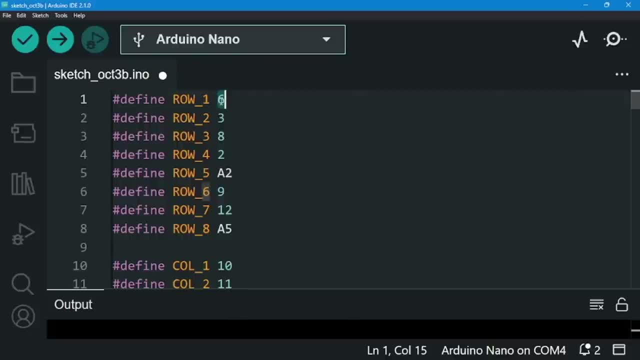 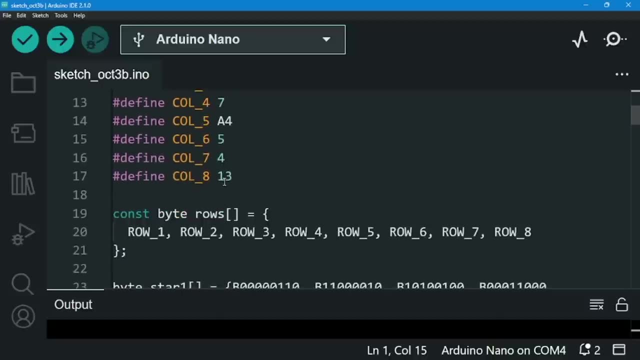 pin 5. right here, if you set it to pin 5, you're going to say pin 5 minus, set the pin 6, so I'm not going to touch it. you're going to be defining your rows and columns and what pin they're connected to. okay, okay then afterwards. 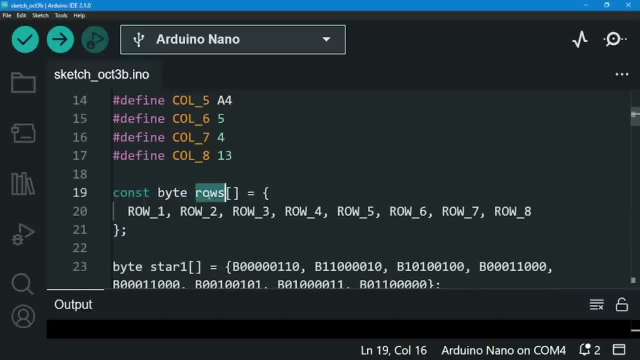 what you're going to be doing is defining the rows, and this one again is going to be written itself. it's going to be preset again when you again like, uh, when you check for, when you check the code in the link below. so don't focus on this, because it's very complicated. 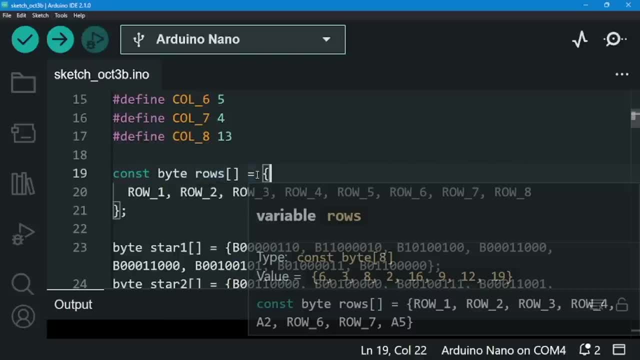 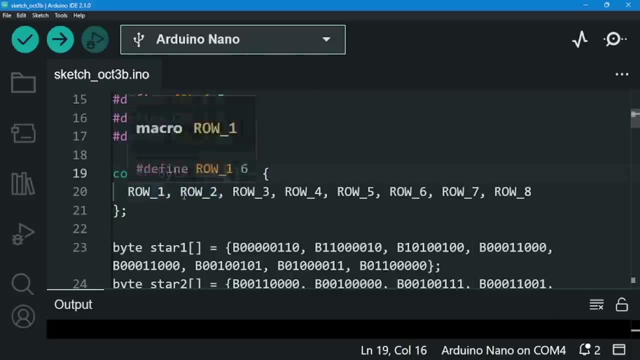 too much on this, but what this does is basically, it's an object. okay, i just want to go over it. so this is an object. that's again, contents what. this is a list that contains what. it's a list that contains what? row one, row two, row three, row four, row five, row six, row seven, row eight. 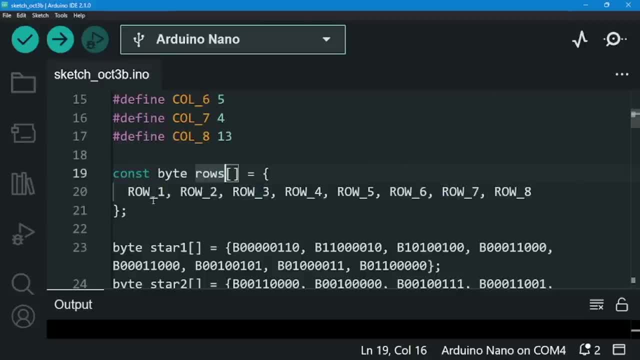 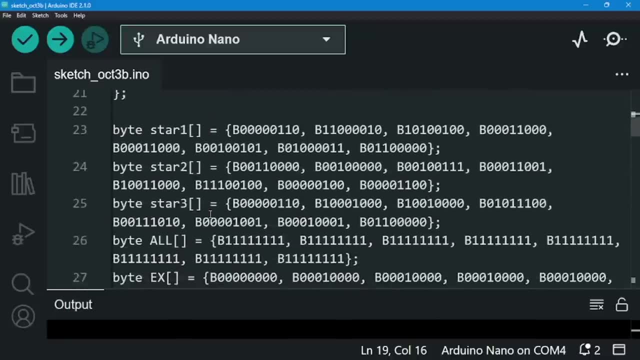 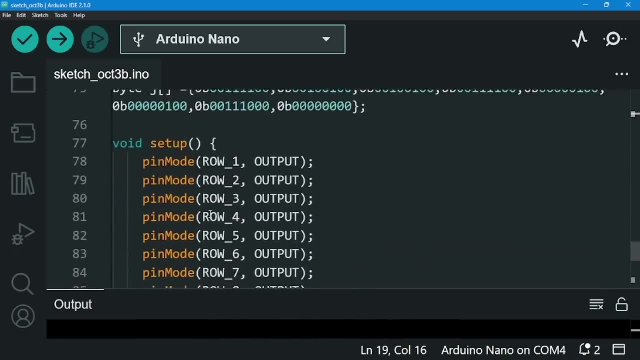 that's what. add a list, add a single list. okay, so it's just listing what, what rows we have here. basically, the ones that are right here. okay, all right, the variables that are right here. let me just skip this right now i'm going to get back to this. okay, and right here, what is very, very. 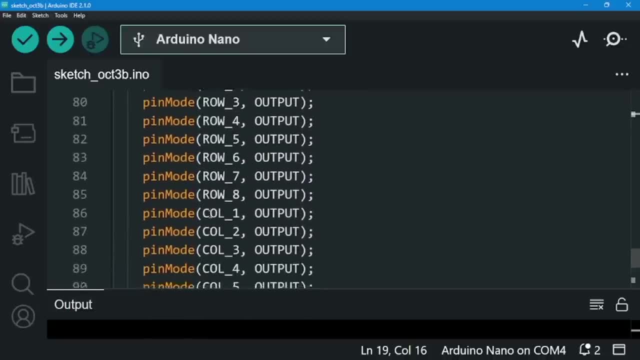 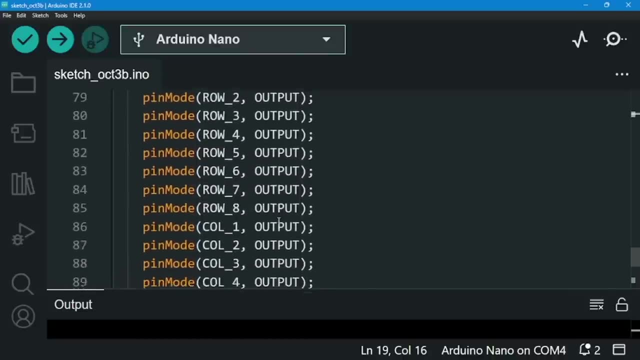 important for you guys is: okay. what is very, very important right here is, again, we're going to be setting the pin mode to what to all of them to output what? all of them to what to an output. that's one thing i want you guys to do. okay, then afterwards? okay, i don't want you to focus on these. 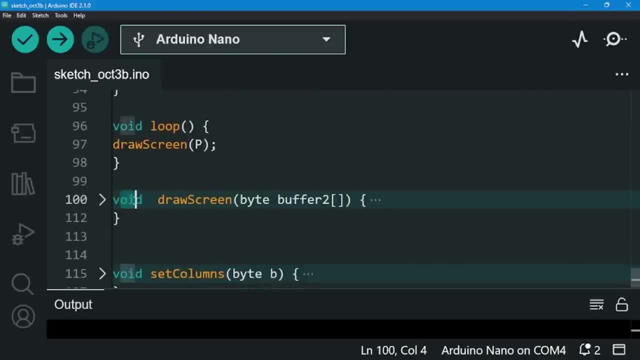 two codes. okay, they're going to be pre-written again on the code. i don't want you to focus on them. they're a bit more complicated again, so don't focus on them. okay, just leave them alone as they. as they are. okay, we're just going to be using them as a library. okay, when we use? 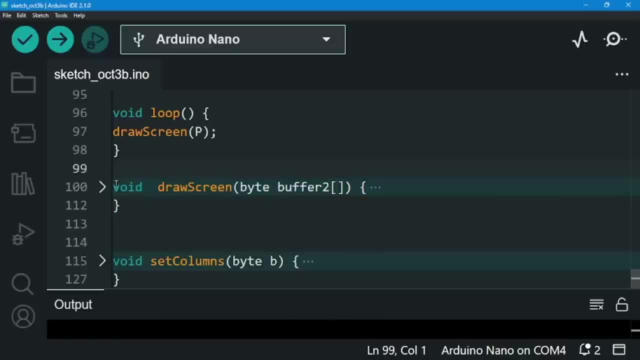 libraries. again, we don't look at what most, in most cases, we don't look at what the behind code of, like how the library works, okay, we don't do that. what we do is what we use, the, what the library, what it provides us, okay, so, like that, again, we didn't play the library. so what i did is, again, this is: 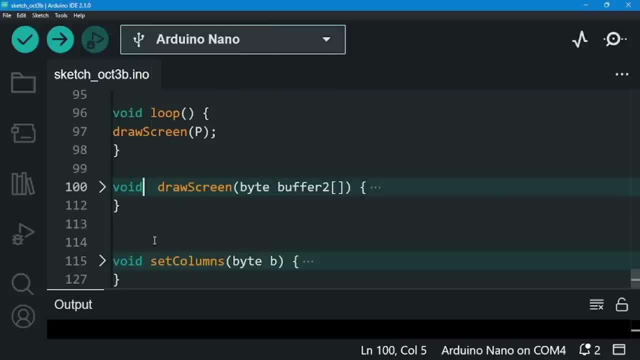 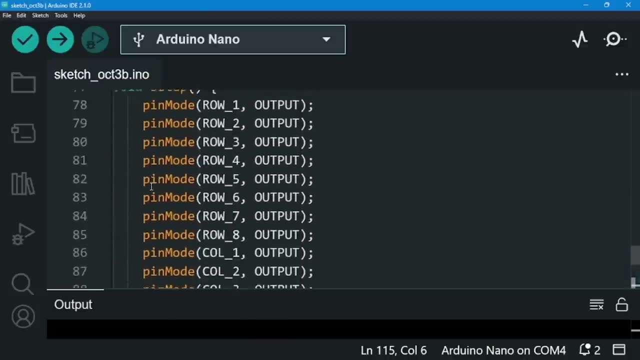 all set up for you guys. so, again, don't focus on these. okay, they're again beyond your scope. okay, don't focus on these. they're going to be written down for you guys. but i want you to focus on is, uh, right here. i want you to focus on this, this, uh, to understand this, what we're first going to do. 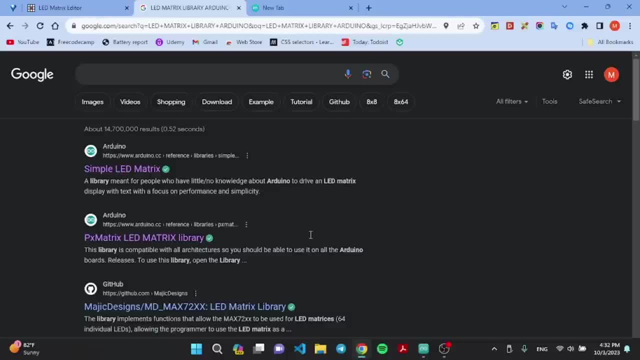 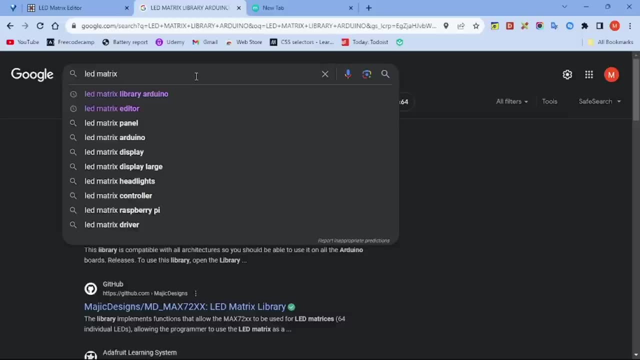 i think for you guys to better understand this is: let me go right here and i want you guys to search for an led matrix- okay, led matrix right here. and i want you to search when you go to led matrix editor. okay, add editor and search for it and then go to: 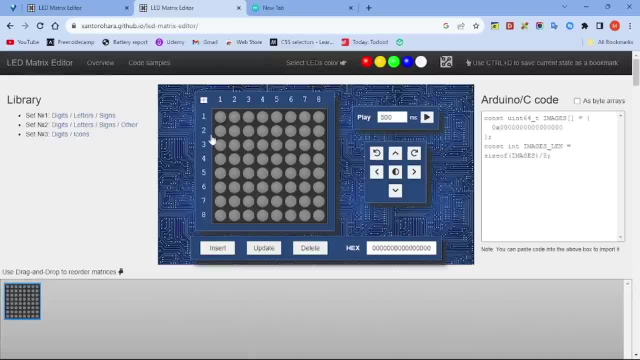 the link right here and then you have your own what digital led matrix? okay, so what i want you to do is right here, okay. what i want you to do is what? it's way better to draw it right here. so let's say, i'm trying to draw l like we did last time, so i just showed you, guys, the. 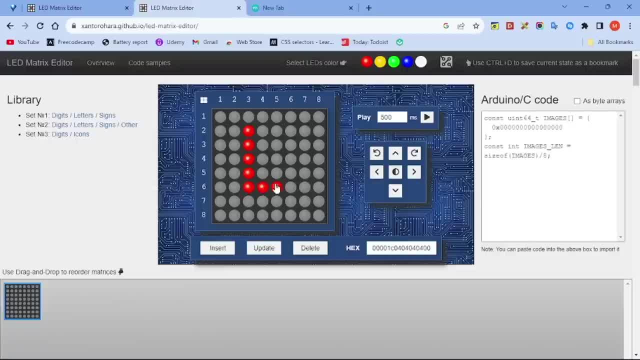 science of drawing an l. so let's try one. let's say we want to draw an l, but the problem here arises is what we're gonna have to, what we're gonna have to first, what we're gonna have to first turn it on before what visualizing. okay, so even to see another right here, what should i do? 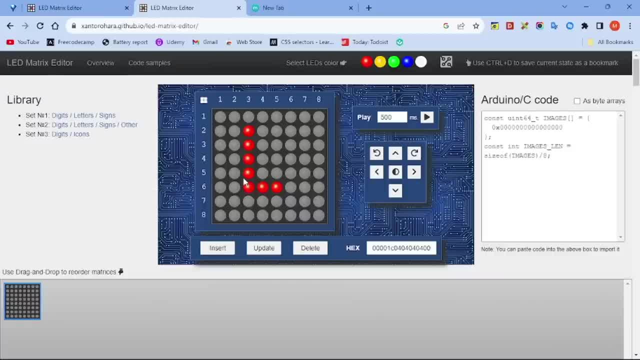 i should visualize it myself before. what before actually, what before actually, what before actually actually turning it on myself. all right, so the problem here is what. the problem here is what we cannot visualize it. we cannot visualize the what, how to draw this in dots. okay, we cannot visualize. 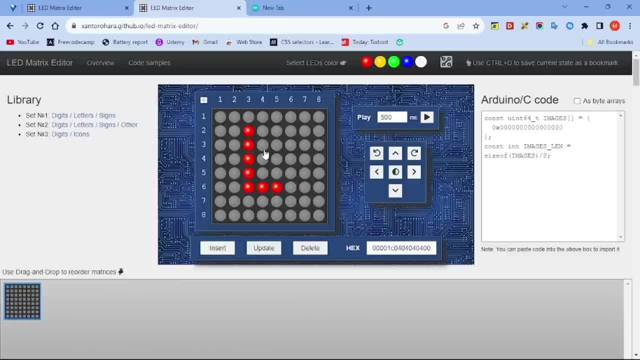 how to draw this in dots, before what, before putting it in our one, in our physical, again led matrix. so what this elapses, what we can visualize how an l is supposed to look like. so we can first do is okay. so what i need to do is like this, then i can know what. okay, i need to turn on column three. 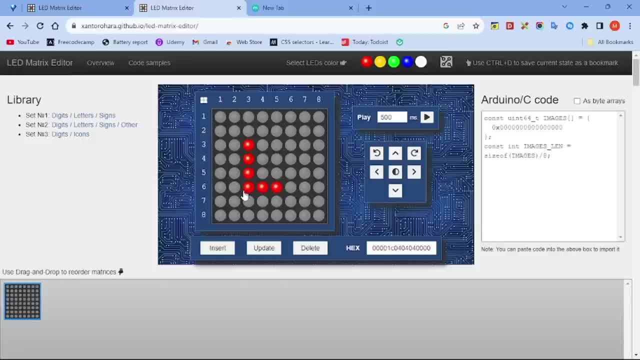 and then- and i'm going to turn on row four, row five, row six- and then, after i'm done with that, what i'm gonna be doing is: okay, i'm gonna be turning this off, i'm gonna be giving it a delay time, maybe a five second, five milliseconds- okay, not five second, five milliseconds. and then i'm 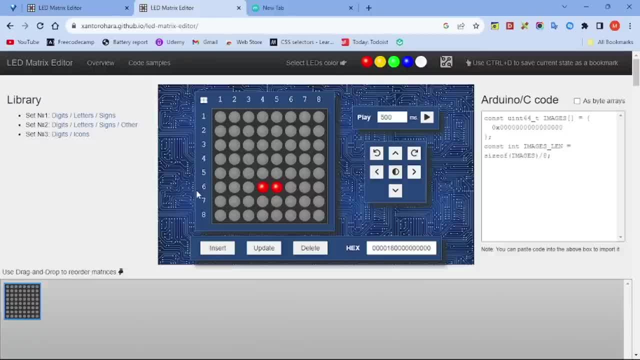 gonna be running this code right here. okay, so i'm gonna turn on row what, row six, and then i'm gonna be turning, turning what, uh, column five and column four and column five to what, to low? okay, so i can visualize it. so, before even writing me down again in dots, you can, it allows you to what to visualize. 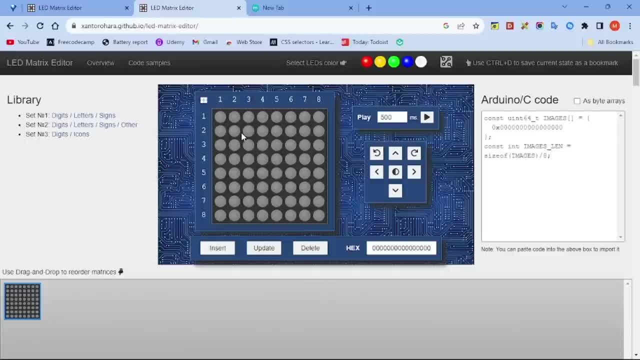 and the best part about this is what? the best part about this is that once you let's say: okay, i wrote down l. okay, let me just write down l or something. let me write down capital l. let me just write it down. the best part about this is: okay, what you're going to be saying is inserting it after you. 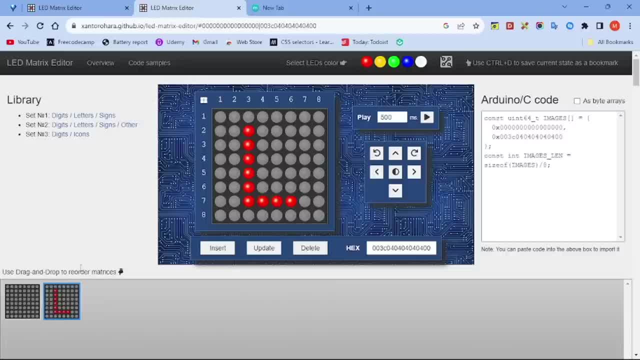 insert it, okay. after you insert the code right here and you can see it right here, okay, and after you insert it, what you need to do is actually delete this. i don't need this one, just delete this one. there we go. once you have again this, uh. 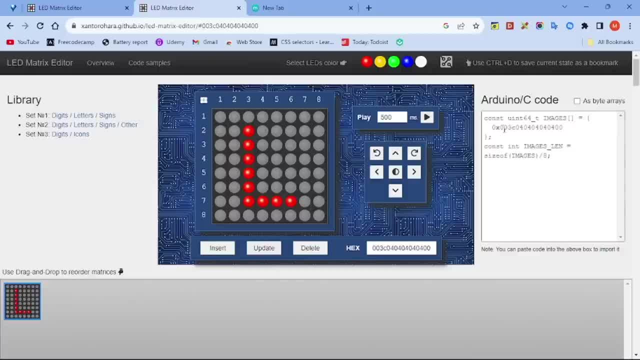 l again. what's the best part is, as soon as you just go right here, the code is written for you. obviously you cannot understand what this is, but as soon as you just touch as byte erase, it's going to change it for bytes, for bits of data, okay, as a byte. once you do that, you can get this code right. 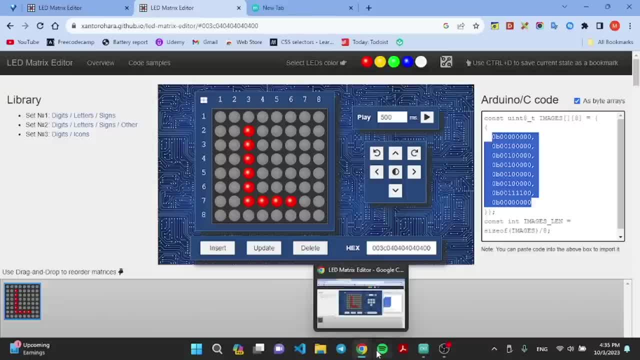 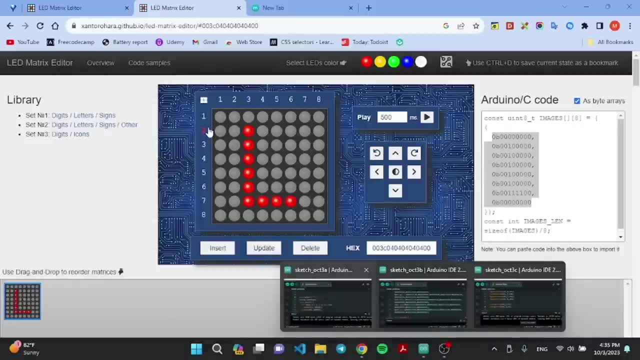 here so you can just copy this and then what you can just basically do is paste it, okay, to your code, basically directly, without without yourself doing it again, without yourself saying okay, after turn on three, and then what two to low, and then keep on doing this and this and this is gonna what involve a series of steps. okay, just not to do that. 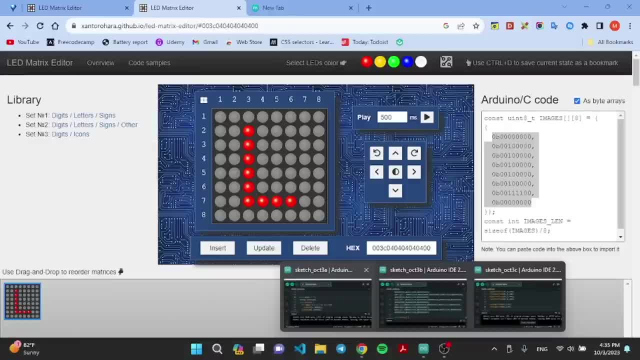 what you need to do is what. what you need to do is only use this in what? in bits? so first things first. let me try to show you guys what this means. so let me just analyze one of these codes for you guys. so i think it's better that way, okay. so right here, let me start. right here, let me start all the. 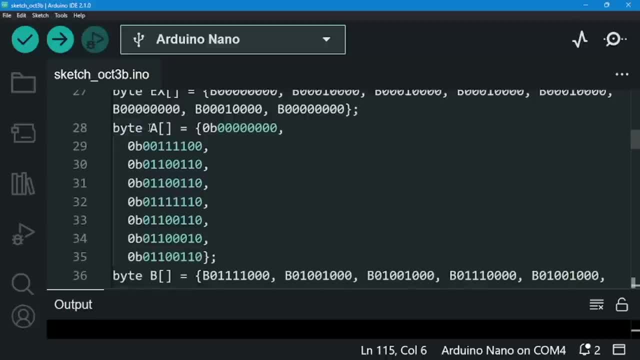 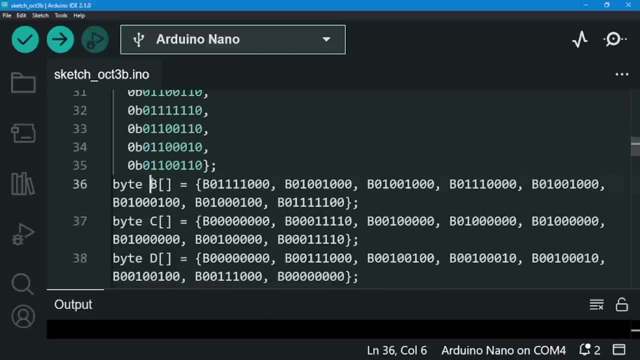 way to the top. okay, there we go. we have a right here. can you see a? can you see a? okay, let me start right here. let me start all the way to the top. okay, there we go. we have a right here. can you see a? a is a bit of a. the code is not right because i was messing around with it. i remember that. 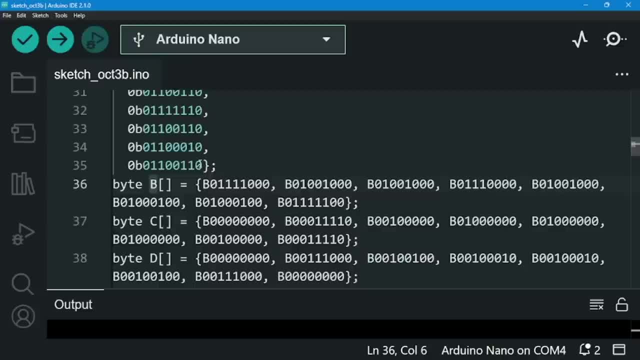 so i'm gonna fix it, though, on the, on the description code, i'm gonna be fixing it on the on the final code. but right here, let's see b, right here. okay, i think b is something interesting to analyze. so what does it do? it says b, okay, byte instead of byte. a byte is what a byte is basically. 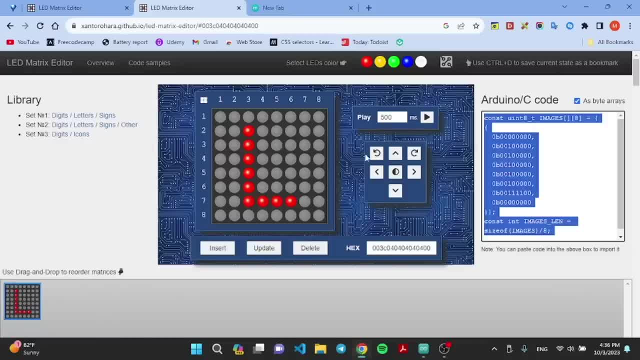 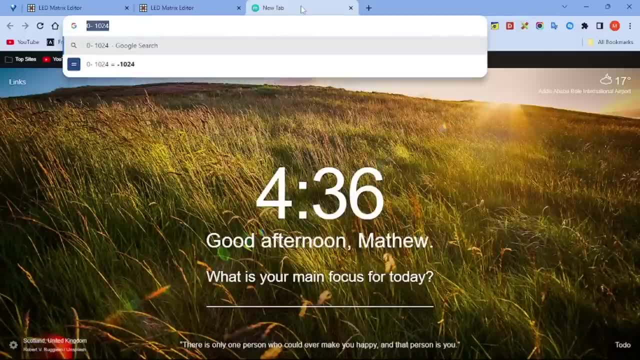 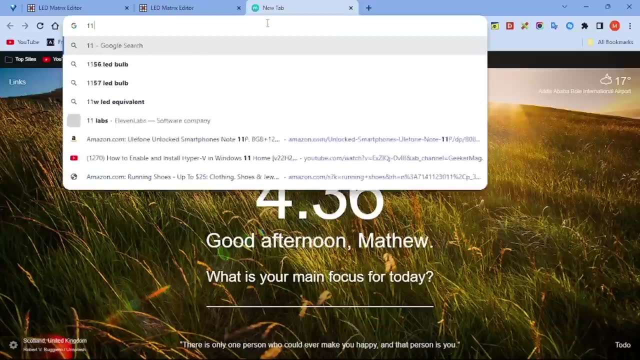 eight bits, just like how we were using again, uh, the number from zero to ten twenty four. remember numbers from ten twenty four, basically these numbers from zero to ten twenty four, they were what they were: eight bits, okay. so basically, for example, ten twenty four and eight bits were in a byte. it's basically what one, one, one, one, one running down eight times okay. 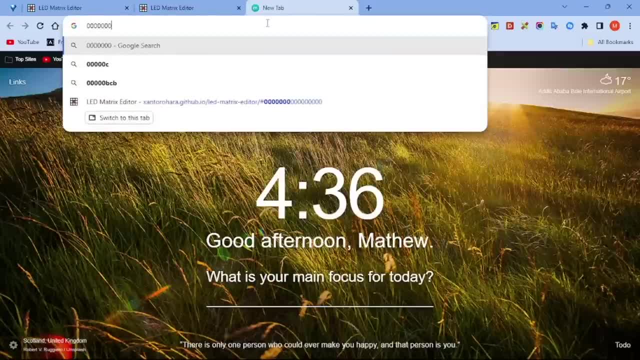 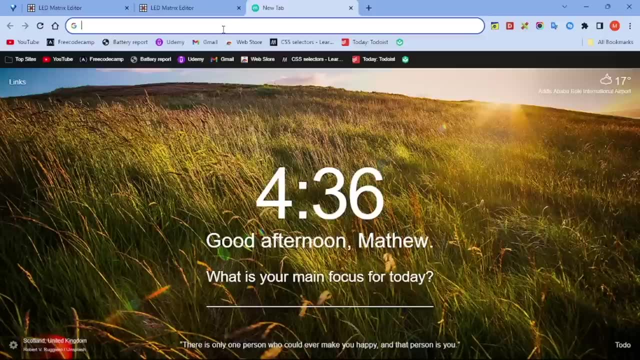 when it comes to zero, what was it? it was zero running down eight times and obviously ten zero to ten, twenty four again. the values again are going to be converted. okay, that's basically what it is, okay. so again, we've discussed earlier. we've discussed about what. 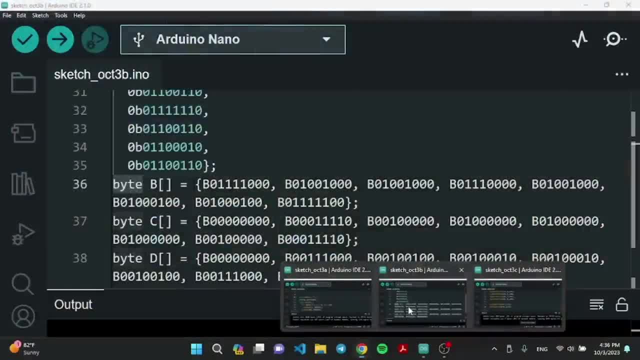 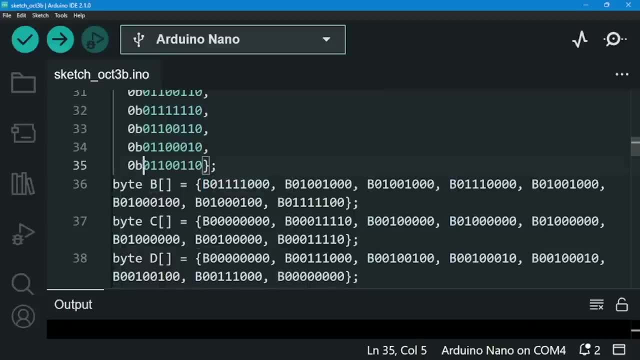 binary. so this is basically binary, okay, okay. so what you do is b and what do they have is right here is a b. they use a b or a small b right here to define what we're telling our arduino. we're not just setting down random numbers, we're setting down what we're sending information and what we're. 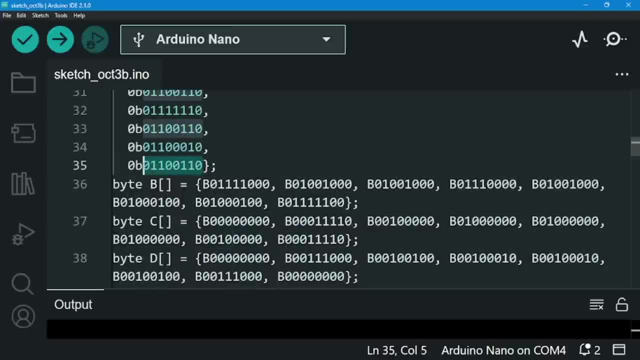 sending information in bytes. okay, we're sending our information in bytes. i want arduino to know that. so you can use what zero b with a small b, or you can use capital b right here. okay, what do you do right here? this, this defines every column. okay, this defines every column. 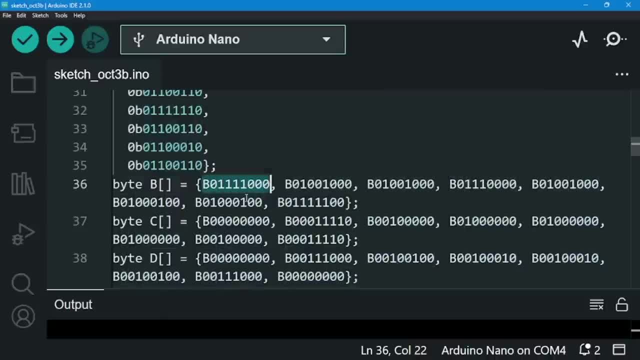 so this is going to be for row one? okay, it's the first one in our list. this is the first one on our list, so it's going to be what? row one? okay, this is going to be row two, this is going to be row three, row four, row five, row six, row seven and then finally row eight. okay, so right here what we're. 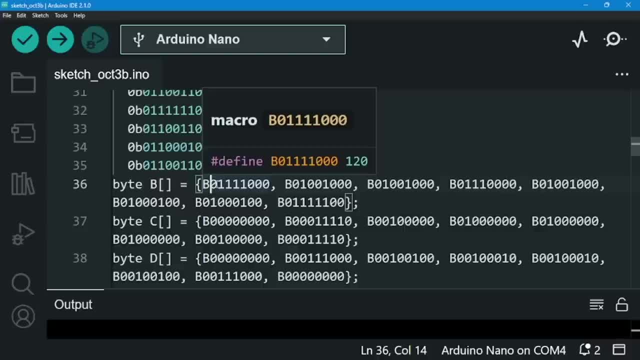 telling is okay. i want you to turn on what. i want you to turn on, row one. i want, i want you to turn off what row one. i don't want to use what. when you set it to zero, it's basically up. i don't want to use what row, sorry, column one and what. i don't want to use column one. 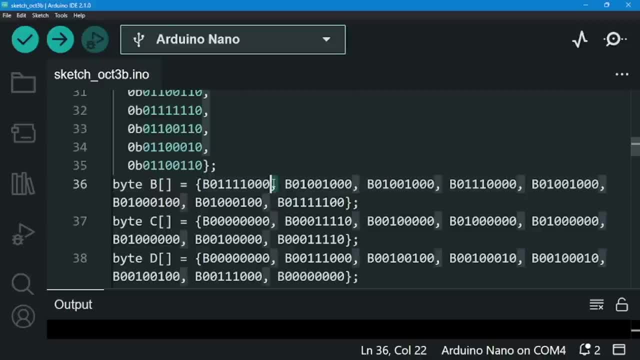 for row one. we're setting this up, okay. this is again the whole thing. is what the whole code right here again, the whole thing is for row one. okay, i want you to keep that in mind. so every bits of zeros and ones is what every bits of zero and one is what, every bits of zero. 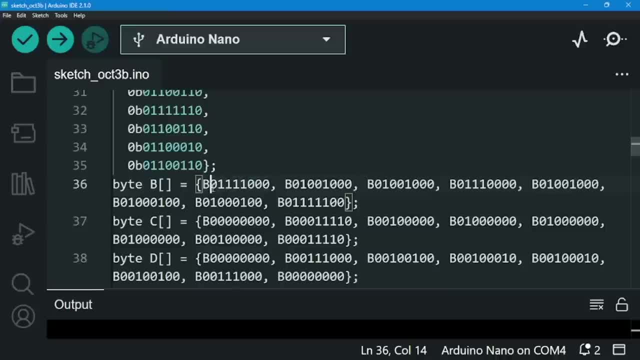 and one is columns. okay. so right here i'm saying: is for row one, i want you to do for row one is: i want you to what? i want you to turn off what column one, basically, what? basically, i don't want it to light up, okay, i don't want it to light up, okay. when it comes to what column two. column three: 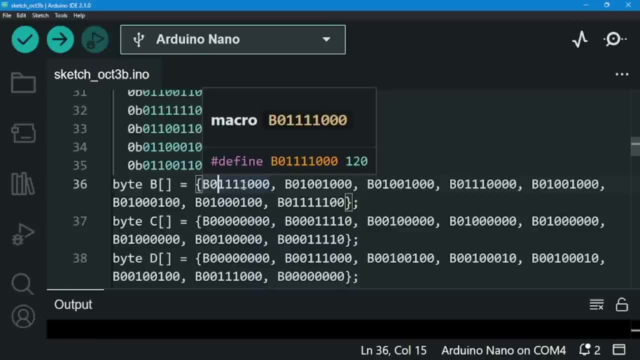 column four and column five. i want you to turn it off. okay, basically what it's gonna light up. i want you to light up what column three, column four, sorry, column two, column three, column four and column five. when it comes to column six, seven and eight, i want you to turn it. what to turn it? 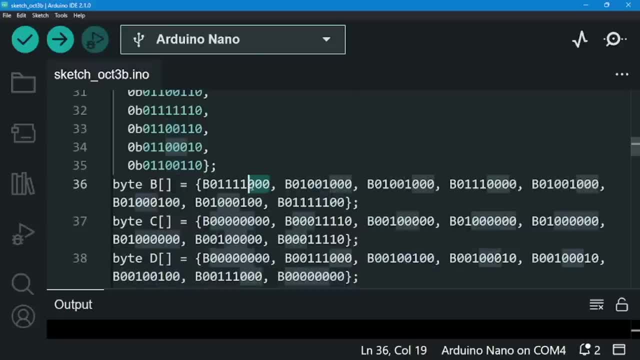 off. basically what i don't want you to light it up. okay, that's what it's basically saying. okay, so, right here, i want you to to do is what i want you to turn on, what i want you to turn on column two, three, four, five. let's try to do that ourselves, right here on the editor, so we can see it ourselves. 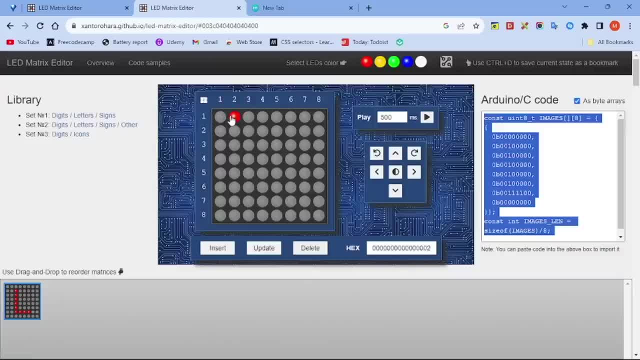 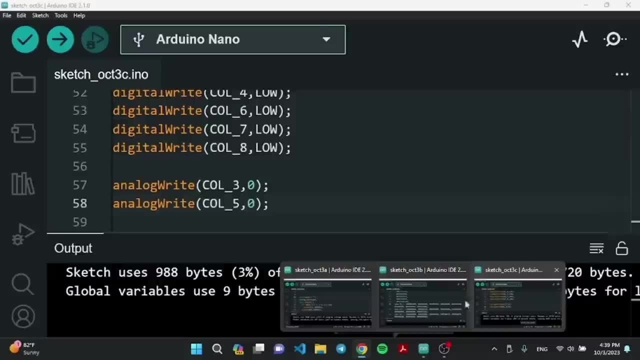 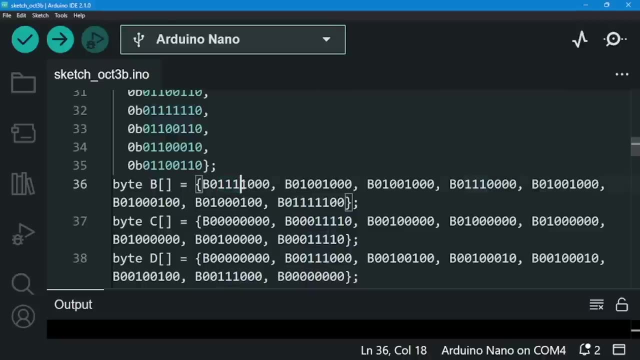 so let's try to turn on- let me just clear this- let's try to turn on column two, three, four and five. okay, for row one. so let's go back to our code right here so that we can understand what this is. okay, there we go. we again define two, three, four and five. all right, then afterwards for row. 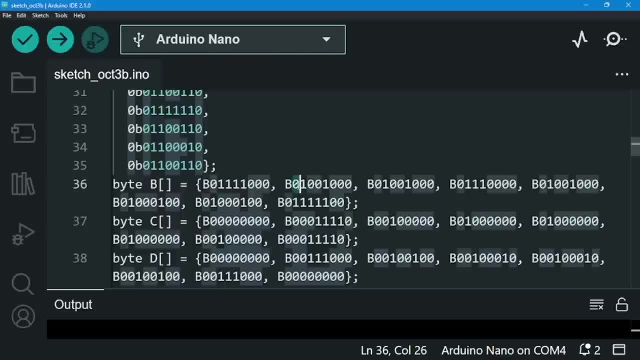 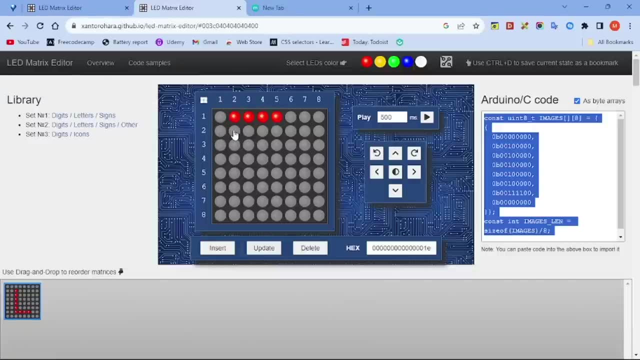 two. what i want you to do is i want you to turn off what column one and then turn on what column two. let's turn on column two right here. column two is turned on on row two. we're going to be turning on column two. let's visualize what's going to happen. let me go back to my arduino right here. 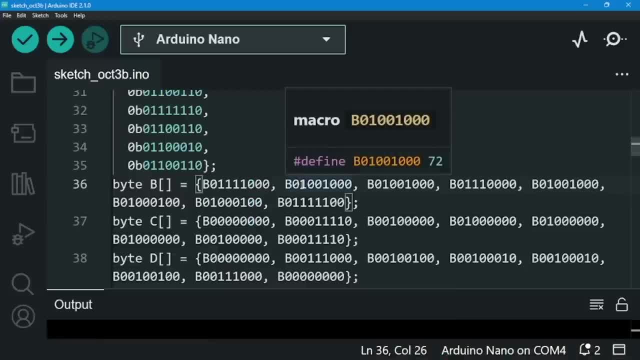 no, it's the other code. let me go back to the other code. there we go, and then i want to turn on. turn off what column? this is column three, four. i want you to turn it off. and then, finally, i want you to turn on column one, column five. let me just count it. let me just count it, let me just. 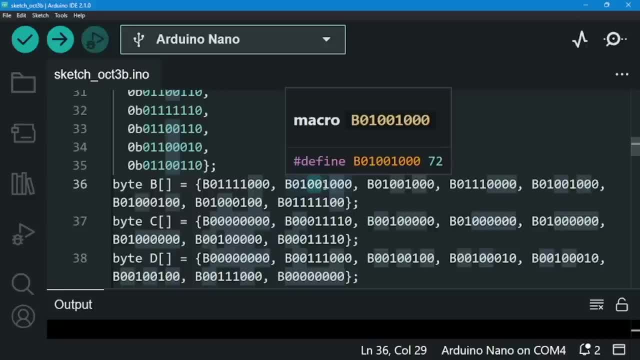 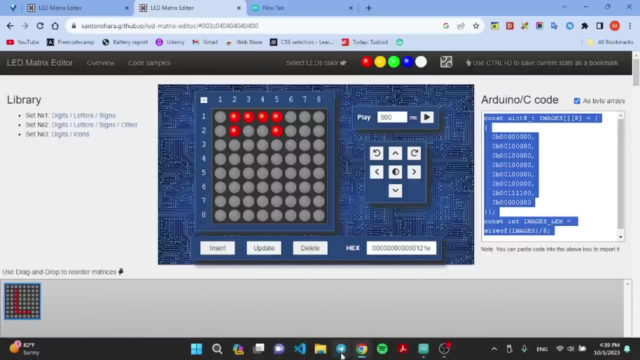 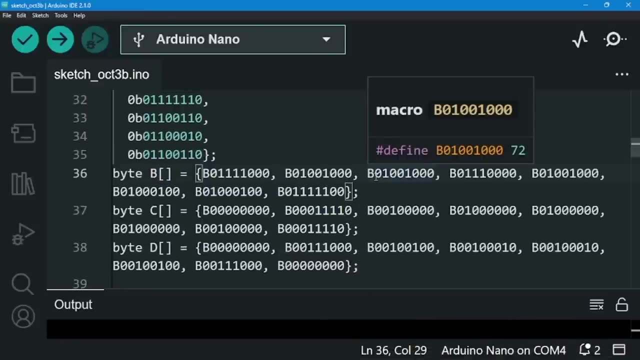 let me just see if i'm correct: one, two, three, four, yes, so i want to turn on column five. let's just do that. let's go back here and turn on column five. there's five, and then let's go back to our arduino code. we're just going to analyze it again just to see how it works, and then i want you to. 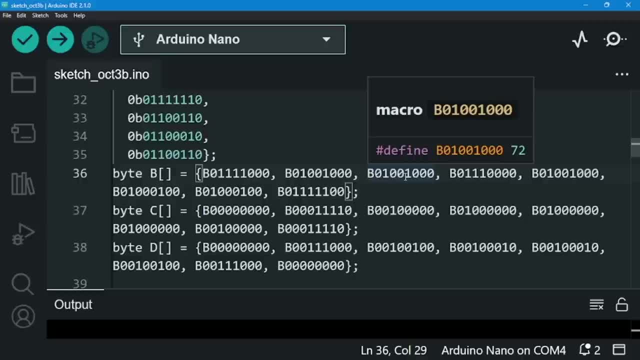 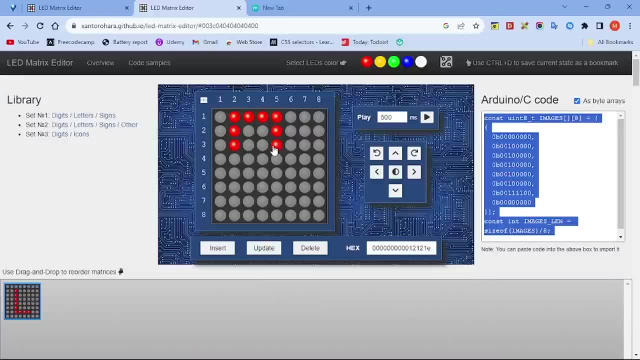 turn on what? column two and column? uh, column five. column two and column five. the same thing as we did right here. i want you to turn on column two and column five. okay, for row three. i want you to turn on column two and column five. all right, i just did that right there. let's go back to our 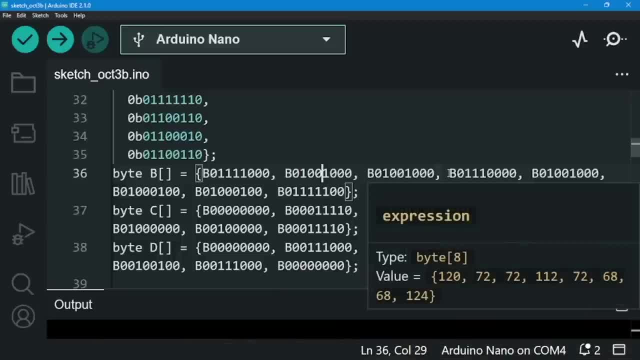 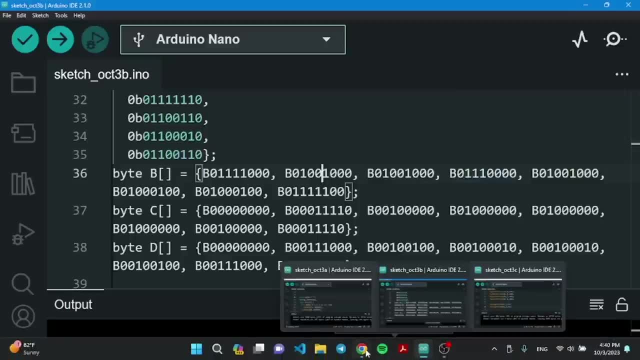 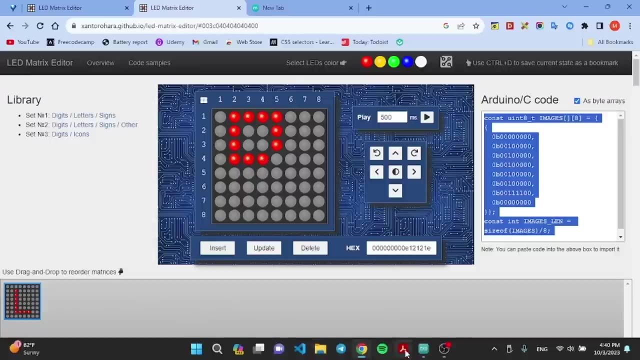 arduino. then afterwards for row four. i want you to do is what i want you to turn on: column two, three, four. okay, column two, three, four. let's just keep that in our head: two, three, four, two, three, four. there we go. and then what do i want you to do? right, here, we read it. okay, we read what? row one, row two. 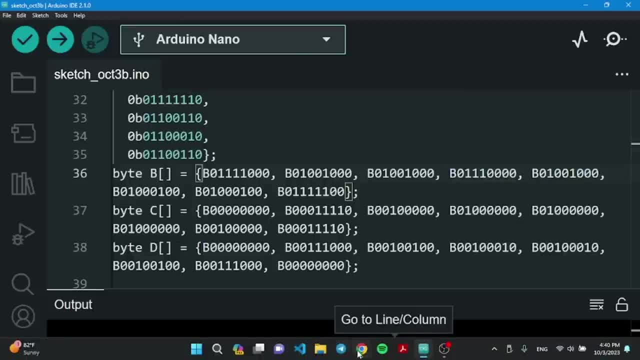 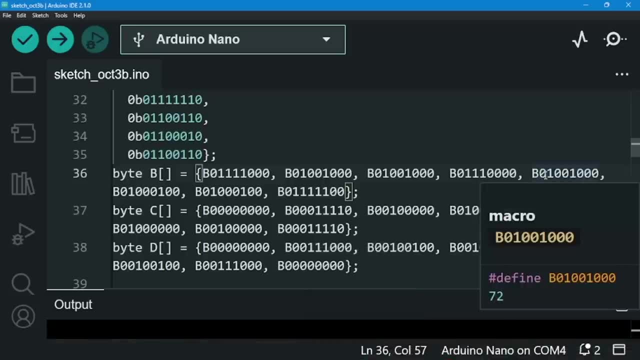 row three. row four: we're on row five right now. let me just check it again. yes, we're on row five. there we go. row five is here. okay, now what? i want you to turn on column two. and then what? column two and column five? again okay, i want you to turn on column two, column five, just like how we did for row two and row. 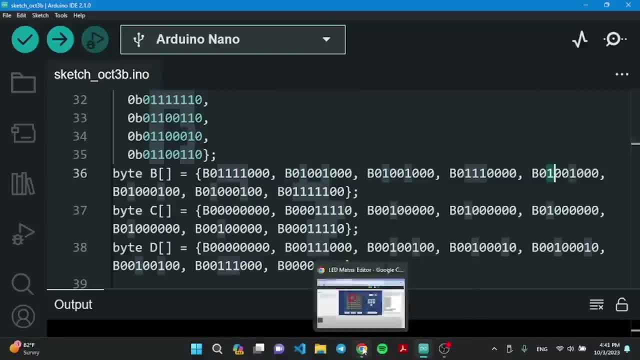 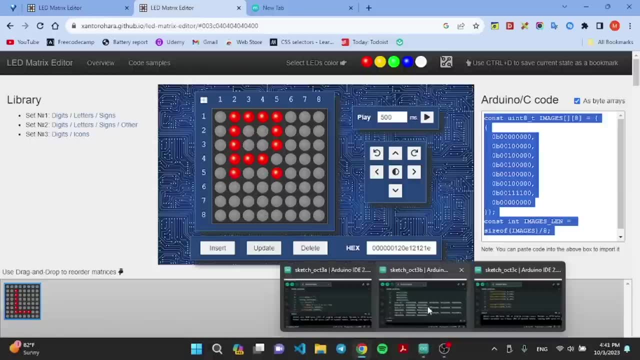 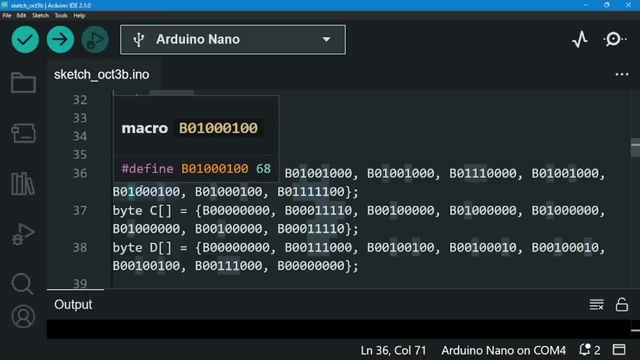 three. okay, so let me just do that. column two and column five. column two supposed to be here and column five is here. there we go, and let's go back here then afterwards what i want you to do. and column, what column? is it column six? we counted column two, three, four, five and then, yeah, column. 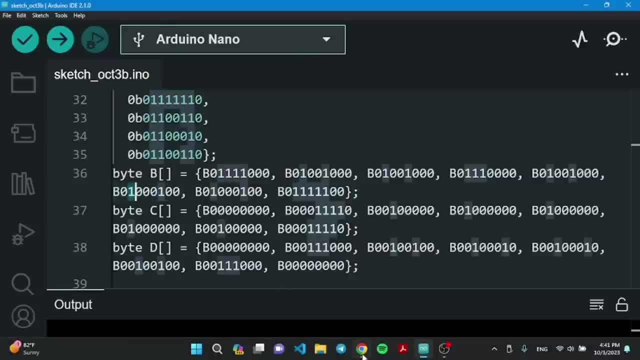 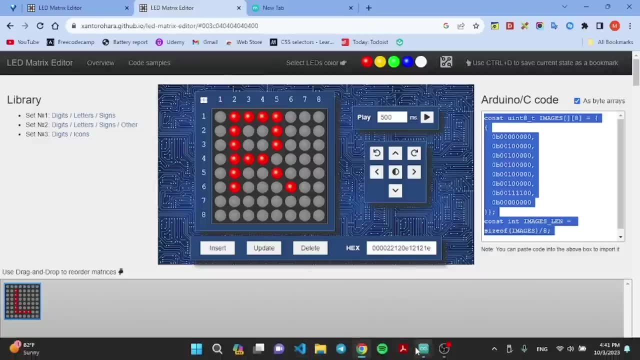 six. so i want you to turn on what? column two and column six. okay, let's just do that right here. column two and column six for row six. column two and column six. all right, it's looking something like an r right now. let's finish it up, so hopefully it's going to appear as b. there we go. i want you. 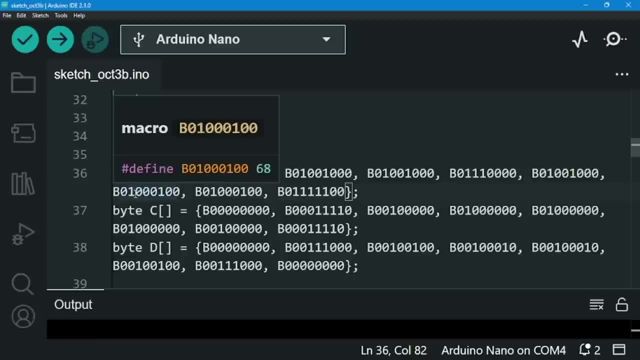 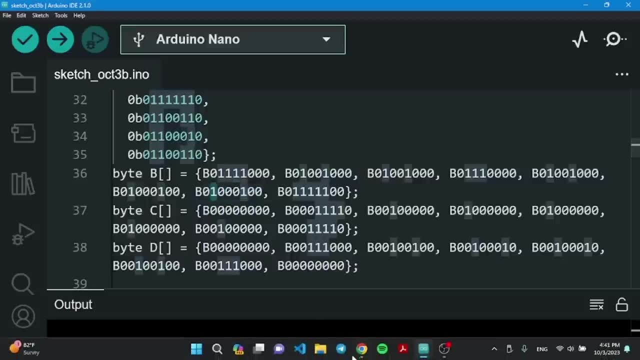 to do is what? the same thing. i'm correct. it looks exactly the same. let me check it. yep, i want you to do the same thing. let me just check it again. column two: this is column two and this is column six. so i want you to turn on column two and column six. okay, let's go to column two and column six. 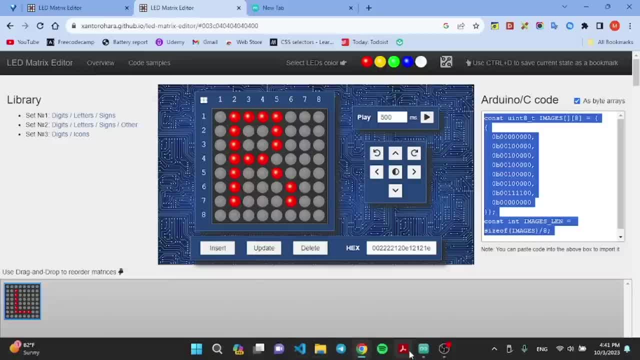 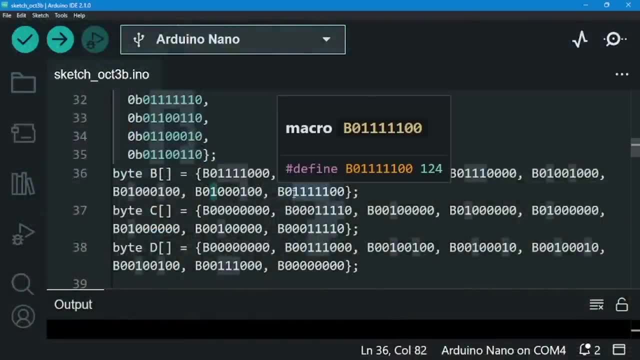 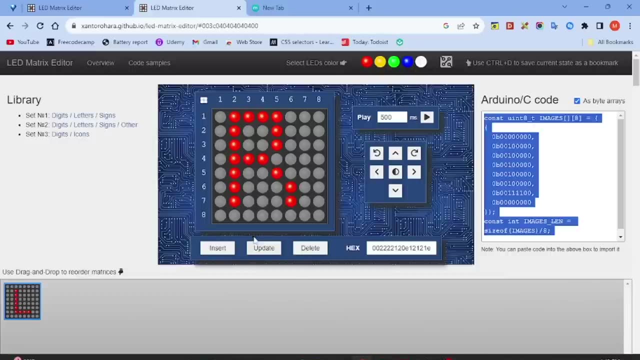 column two, column six. there we go, and then, when it comes to the row eight, let me go to the row eight, right here, the final row. i want you to do what i want you to turn on column two, three, four, five, six. so let me just do that. i want you to turn column two, three, four, two, three. 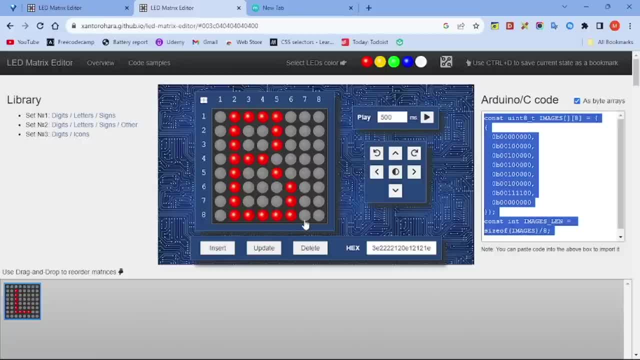 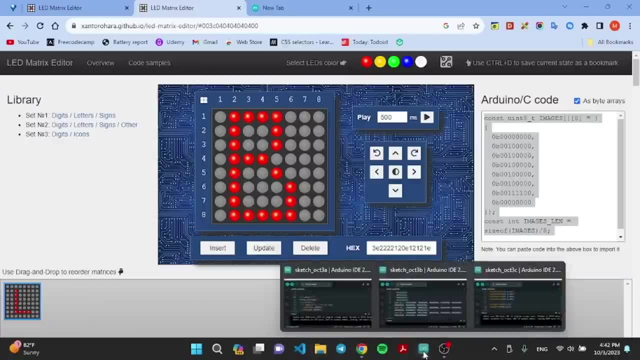 four, five, six and there we go. we have one. we have somewhat of a, b right here. this is basically what's going to draw if i call it, if i tell it to draw b. so what you need to do again to draw something is okay. we have the information again preset for you. have the information preset for you have. 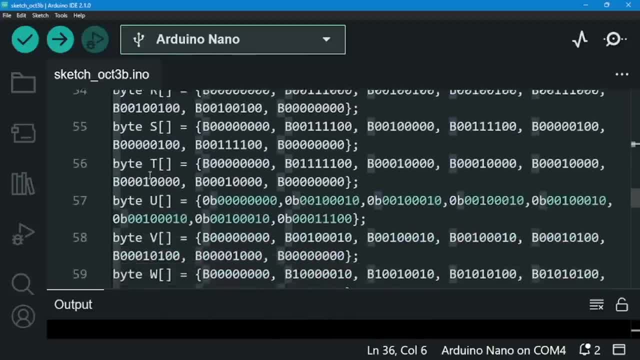 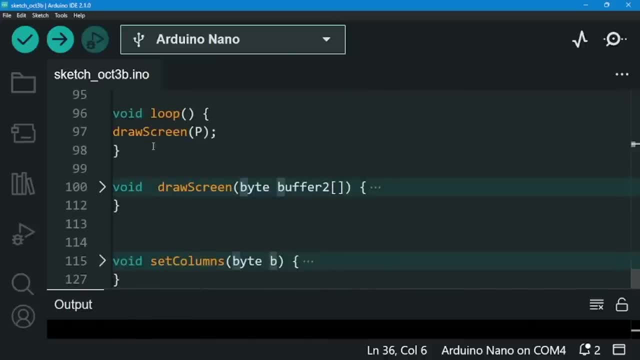 b, right here. c, d, everything from a to z, from a to capital z. i have it written for you guys. okay, from a to capital z is written for you guys. okay. then what i want you to do right here, okay, is you're going to say draw screen and then you tell it: i want to draw a. 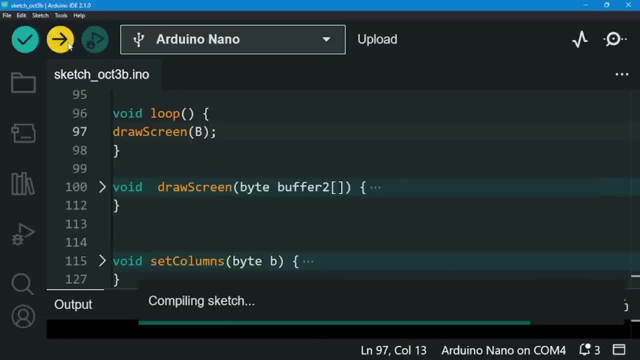 b. let's see what happens right here. let me just upload this. it's compiling and it should be done. uploading, that's all you need to do. i want you to do is what? use the function draw screen and pull what again, what you want to draw, right here, as soon as you set it at bytes: right here once. 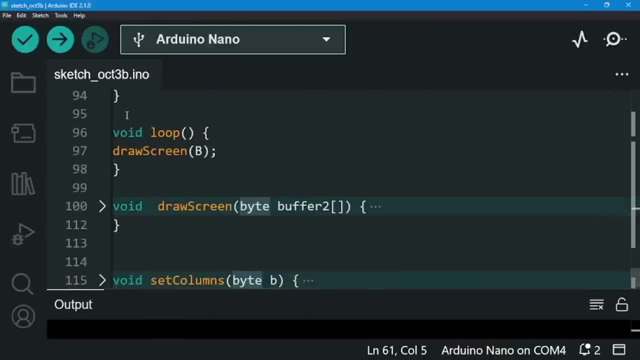 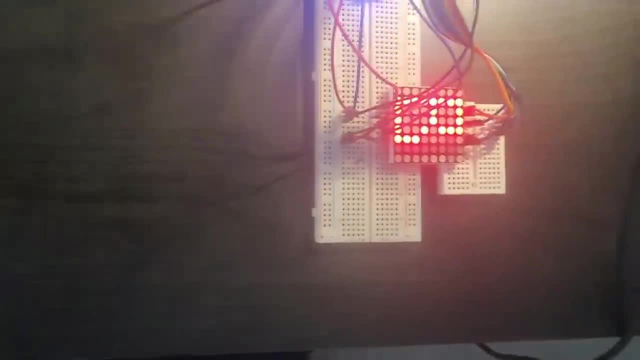 you set it to a byte. what i want you to do is use it. okay, there we go. draw screen b: can you see it? let me just check if you can see it. let me turn off the light for you guys. let me bring this closer, actually, bring this closer. i don't want to touch the wires. they're very, very fragile. i. 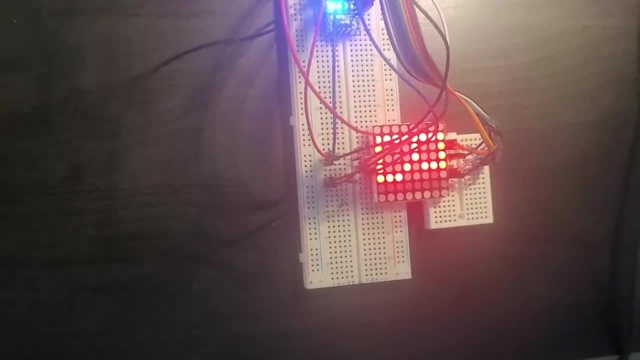 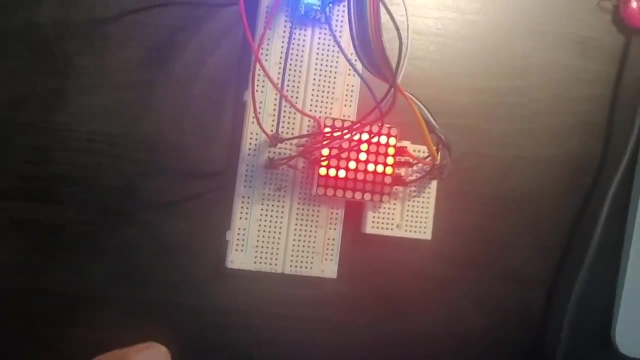 was about to push the button. but i'm not going to push the button. i'm going to push the button away for you guys. but they're very fragile because i can just ruin the whole thing and i don't want to again connect 16 pins. it's going to be a lot of work. let me just go from this angle so you can see. 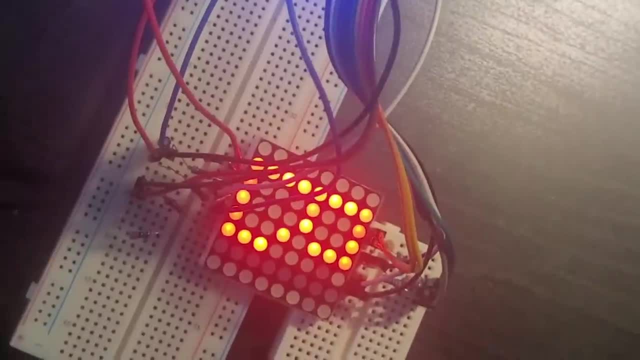 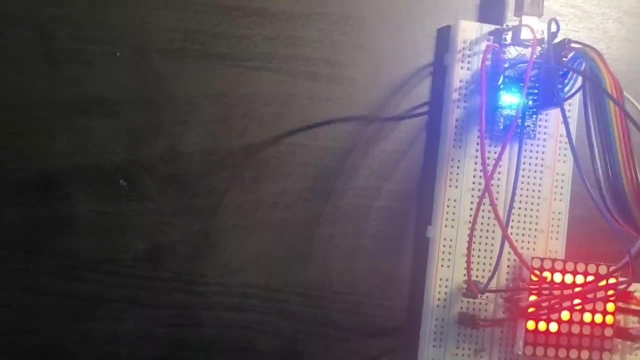 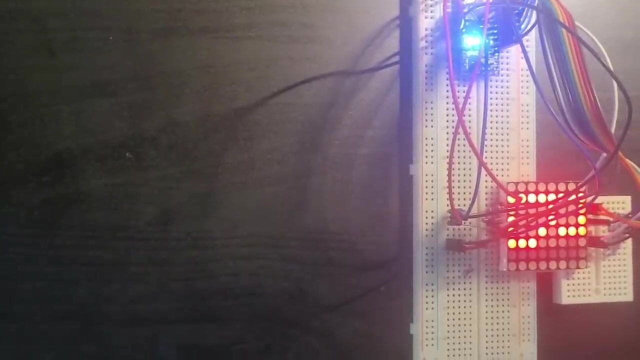 it. there we go. i want you to focus on this. there we go. it's drawing out the b that we just drew on the one on the matrix editor, basically on our what? digital matrix. so let me just zoom this back. okay, that's good, all right. so, right here, we draw b, and i already said this, set this for you guys. so again, 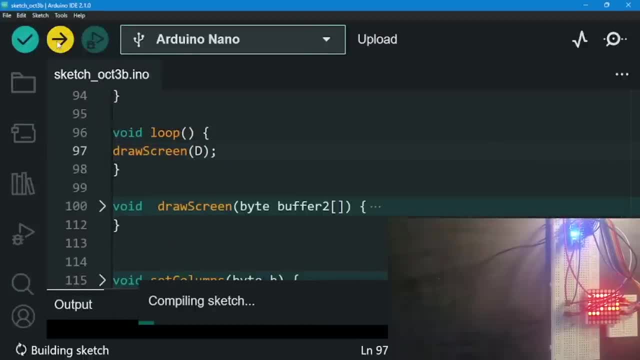 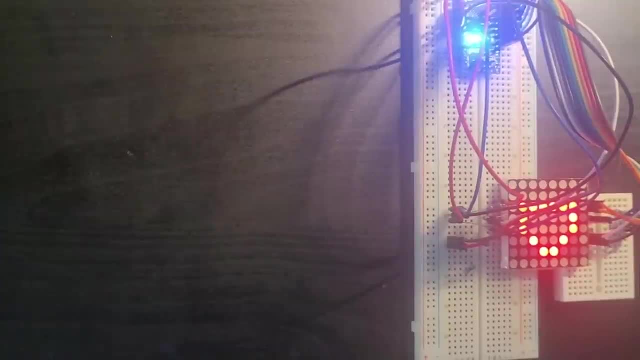 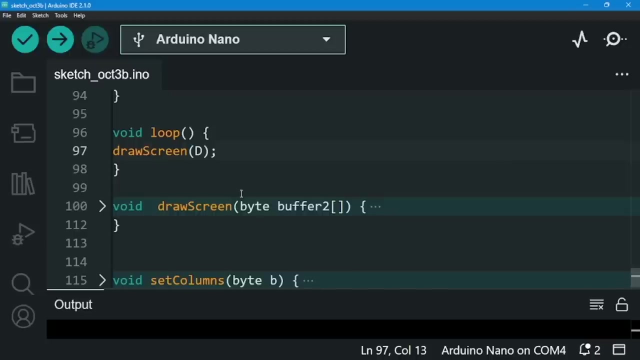 you can write: draw on d e anything you want. let me just upload d right here. let me just: i want to draw d, let it draw a d right here. there we go. we have g drawn out for you guys. so almost every letter is again. i already preset it. so what i want to do here is, again, we can use this to do what we. 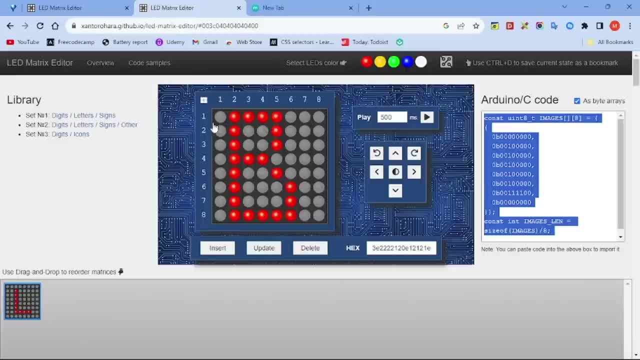 can use this to again set up what- not only letters, we can also use it to even do a simple drawing. so what i'm going to be doing is i'm going to be drawing a simple face right here. i'm going to be trying to draw a piece at least. 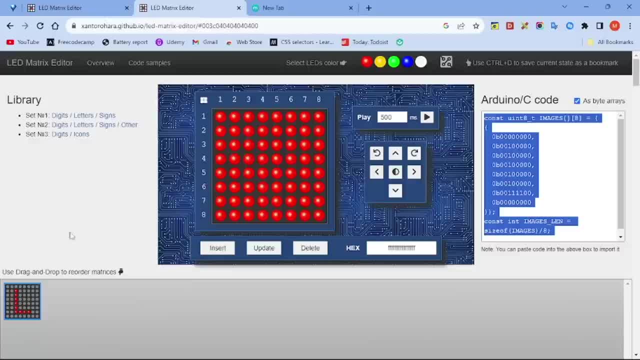 i'm going to be trying to draw a face right here. let me go to l right here. let me delete it. i don't need it anymore. i don't need it. let me just delete it and let me just reset everything. and once i'm done doing that, let me just try to draw a smiley face. not the best drawer, but 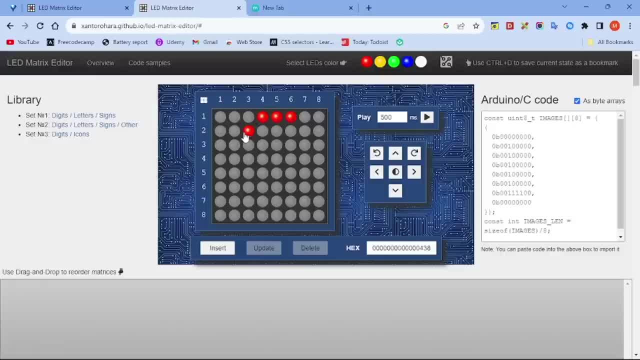 let me just go right here and let me start like this. i think it's better that way. let me just keep on trying. all right, let me go like this and then let me just try to do exactly the same thing here. it's a bit of a struggle because i don't know how to. uh. 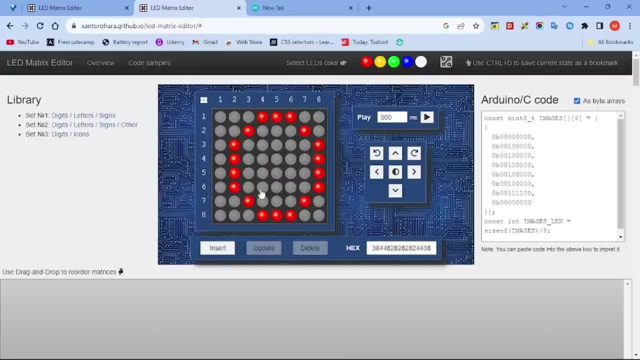 i'm not the best drawer right here. okay, i mean, it's not bad. it looks like a good circle- not the best one, but i think it gets the job done. okay, let me put two right here eyes and then let me just try to draw a smiley face on it. let me just try to do that. there we go. we have what. 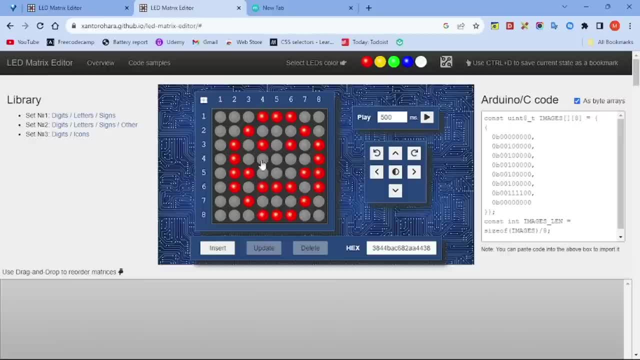 a smiley. what we have a smiley face right here. have a smiley face, so let me do is insert it right here. okay, once you just insert it, the code is already written for you guys. so again, lighting up all of these individual or individual again, um, individual or individual bits of dots would be really hard, because you're gonna have 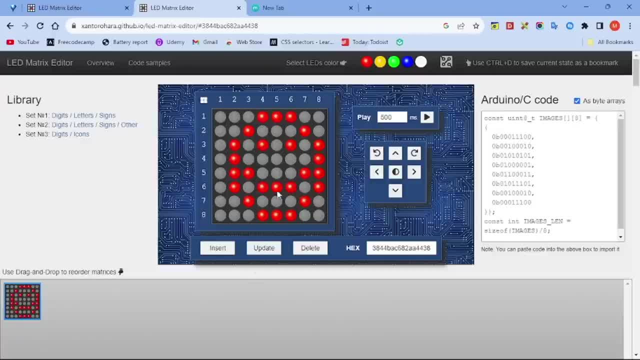 to do a lot of what. a lot of work. just even light this up, just to know which one's which, and if you mess up a one spot you have to go back check everything again. you have to do almost how many we used around. let's say half a fit right here we use, let's say it roughly- 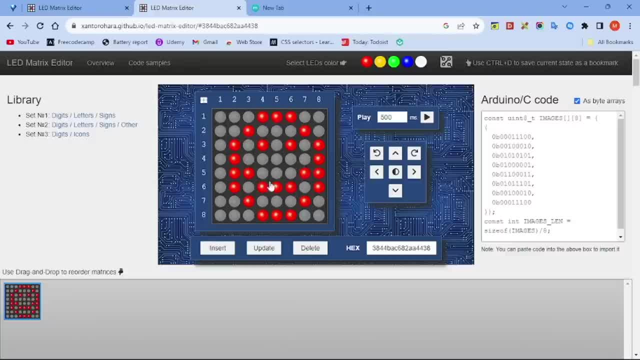 say, uh, maybe a two-fifth of it, two-fifth of the 64 again dots that we have here, 64 bits of what bits of again lights that we have here, and basically, if we just again try to do it physically, again set this to high, set it to low and doing all of that, it would be a lot of work. 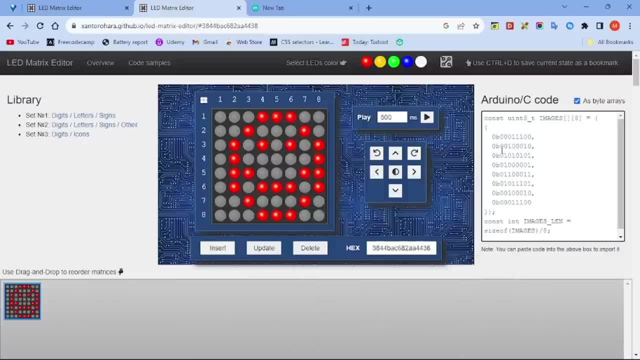 okay, so we're just going to be using this and you're going to extract this information right here. okay, that's all you need to do. once i insert it, the information is out, going to be right here. it's already going to give me the code right here. again, make sure it's written down. 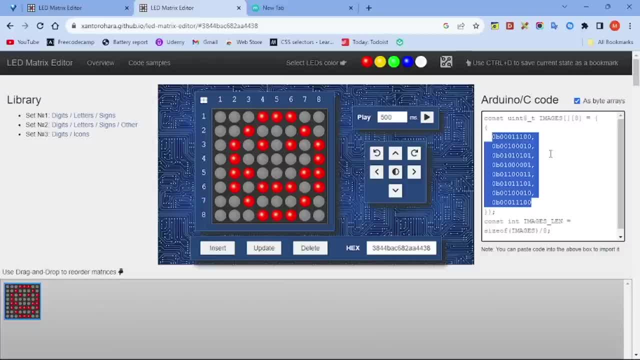 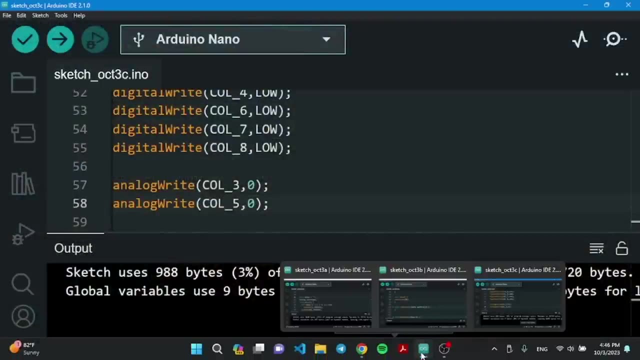 in bytes and byte erases. this is again selected. just make sure that this is selected. let me just copy that. let me just again- let me only get the code right here- copy that, okay, let me just copy that. and uh, let me go right here. oh, not this one, let me go right here. there we go and what i need. 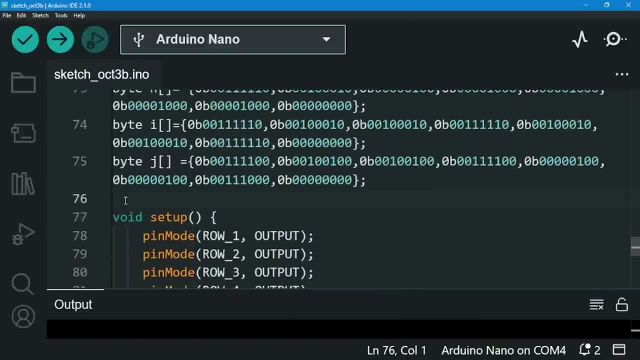 to do is what i added as a byte, okay, as a byte of information. so i'm just going to say byte and i'm going to say let me call it smiley, because this is a smiley face, so i'm going to say smiley face. 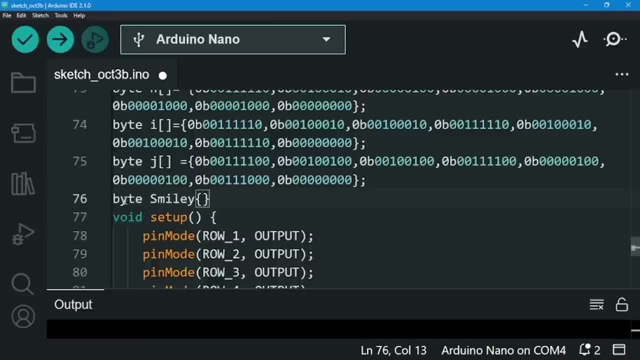 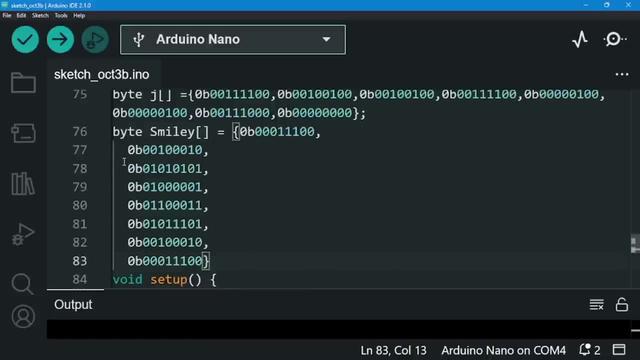 just call it smiley, and then again i'm going to need to again use again what, my, what, my brackets right here just to indicate it's a list, and then afterwards i can paste it. there we go, let me just again. i don't want it to be spaced out, so let me just give it space right here. let me just make. 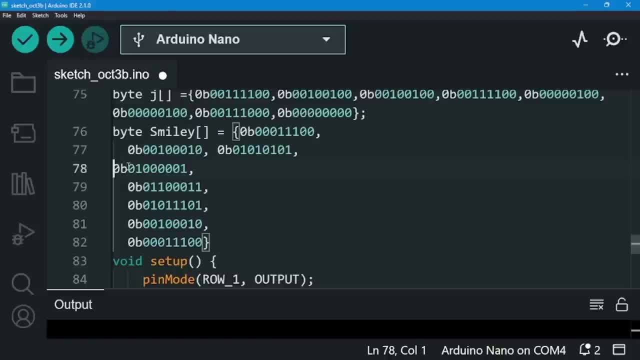 sure that again it can take up a whole line. this is valid, but again, from an aesthetic point of view, every, every, what, every, what, every row right here is taking what a line up. so it doesn't look that good. let me just again, without touching anything, just right here, let me just make sure that i'm 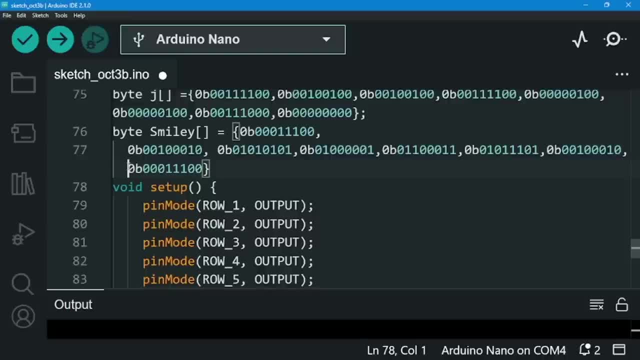 just removing the extra bits of the extra bits of again spaces right here. let me just remove them. okay, i think this is good. okay, i have to remove this one that is here and with the extra bits of again, there we go, the extra bits of spaces that we had here. now this looks better and let 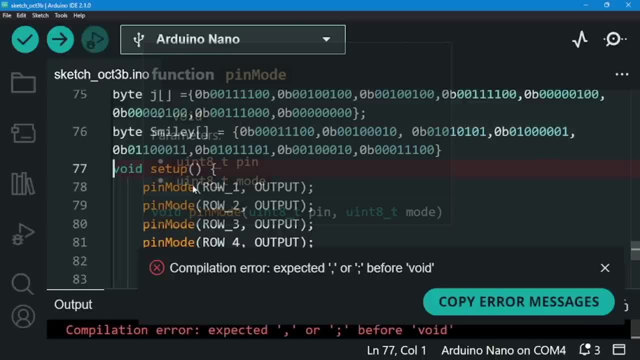 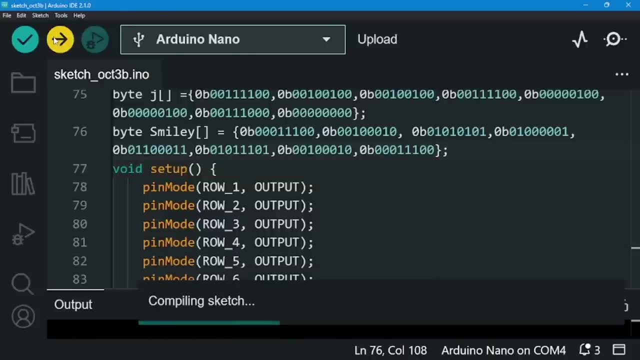 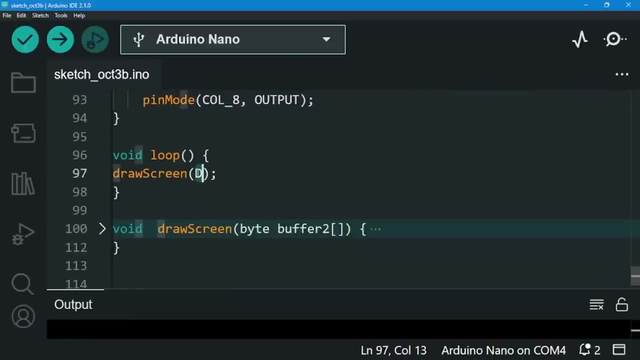 me just upload it right here. let me just upload the code. oh, i forgot to do. i forgot to give it a. what a semi-colon at the end. i defined it right here, smiley, it should be working. it's done compiling, and now what it should be done: uploading. okay, let me go to draw screen and i want to draw. 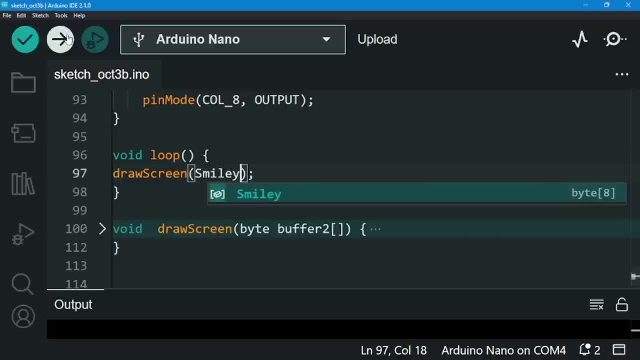 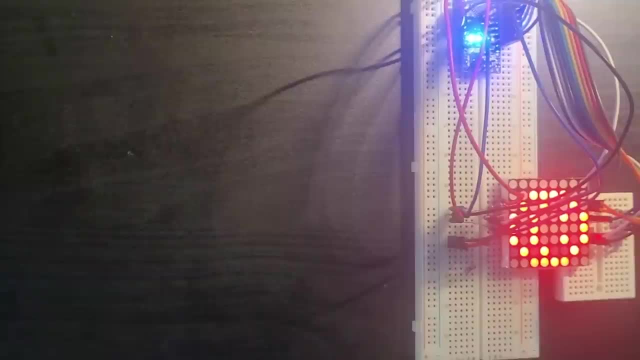 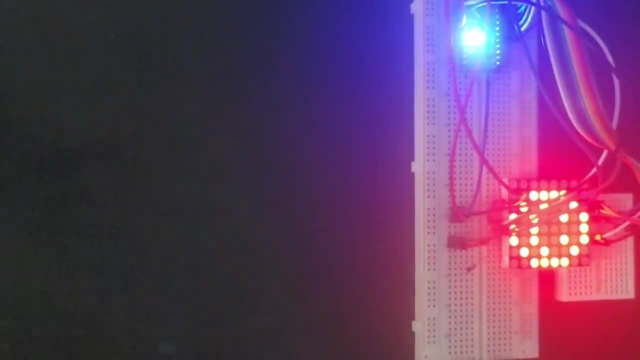 what smiley, smiley. let me try to draw smiley right here. it's done compiling, okay, now it should be uploading. and there we go. we have a smiley face. can you see it? let me just turn off the the other light- not the best lighting, but i just want to make sure that you see it for yourselves. 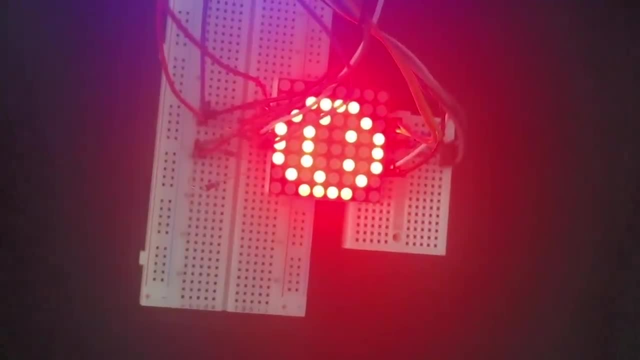 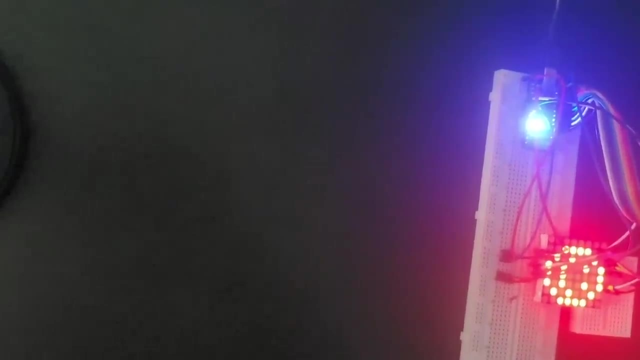 let me bring it closer so you can see it. there we go, we have a smiley face right here. so again, it's up to what, it's up to your imagination, again, to do these things. so you basically can do what you basically can do, and obviously you cannot do everything, but you can do lots and lots of things. 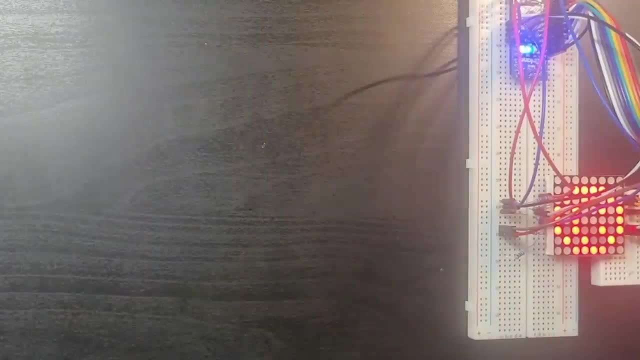 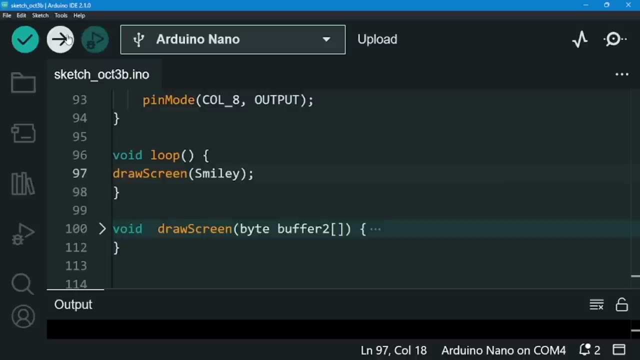 it opens possibilities that were no longer possible, and what that were not possible using a seven segment led display. so what i'm gonna be giving you guys to do is what? right here again, i have the preset code. what i want you to do right here is okay. 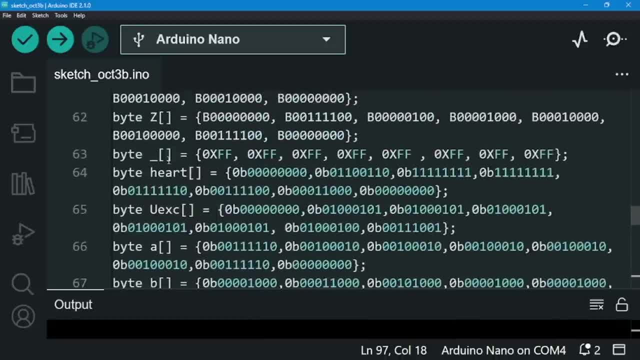 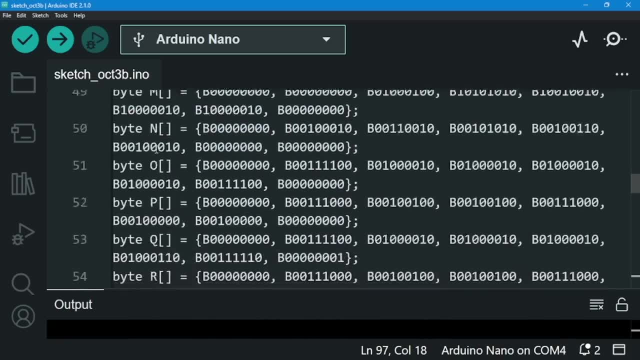 i do not add every alphabet. i added every alphabet, like every capital letter, from a to z, as you can see right here. add it up and just set it up right here for you guys. but one thing i did not do is i did not finish. there we go, where is it? i did not finish writing. 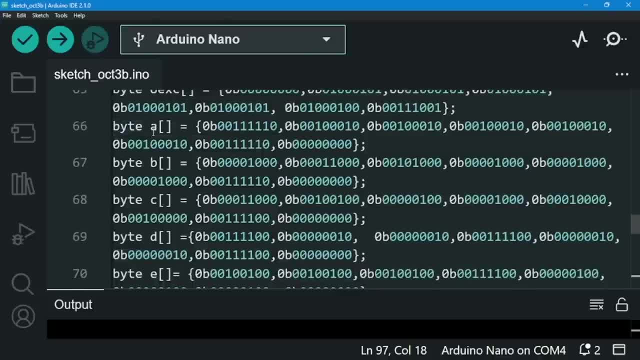 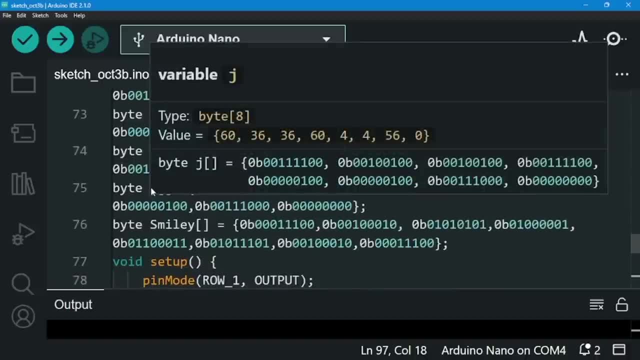 down every small letter. okay, i have a right here, but i did not finish writing down everything. we have a, b, c, d, e and i stopped at, stopped at j. okay, what i want you to do is add up to it. okay, i want you to add it up all the way up here so that it is close to the top, and then you 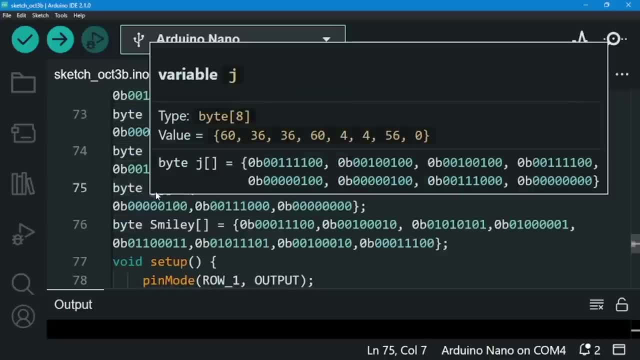 can always go to the top, the bottom, and then when you finish that, you can go back and write on it, or you can go back and you can. will do whatever you do. go head to the top, you can go, and to small c. okay, i want you to add up all the way up to small z. and one important thing: i want you 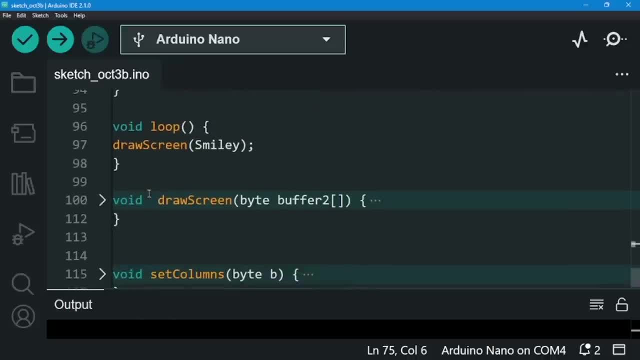 guys to do is okay. again, one thing i want you guys to do is: don't focus off on this code, but what i want you to do is write down a word with it. how do we do that? how do we write down a word? uh, if you, again, what i want you to do is we want to write down a word, how we display a word? okay, 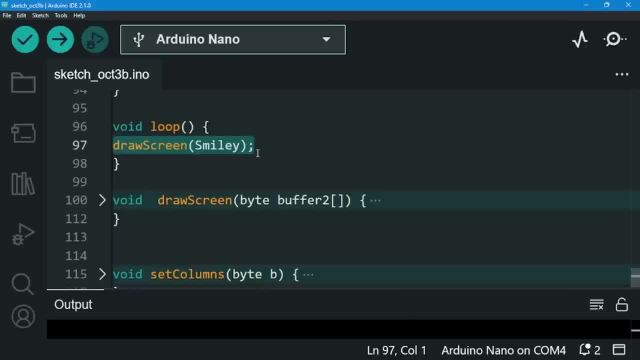 how do we display a word? i want you to think of it. so, again, i want you to pause this video, think of it for like at least a minute or two, and then come back this video where i'm just going to show you again how we just do it, because we've learned this so far. it's going to be very, very simple. 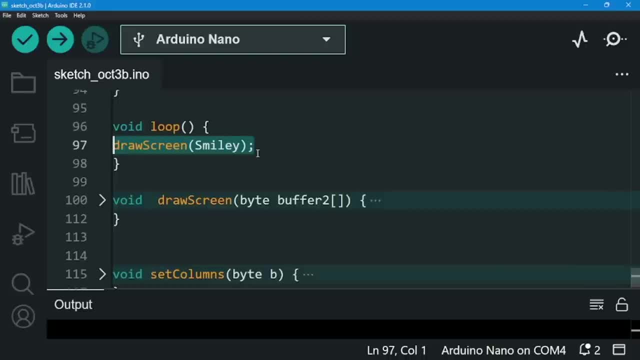 okay. so i'm just going to be waiting and hopefully now you have again resumed the video and then hopefully you got it right obviously to to write down where it's there, what they're just a bunch of, what they're just a bunch of letters. so what do we need to do? let's say i want to say the word arduino. okay, how do i do that? 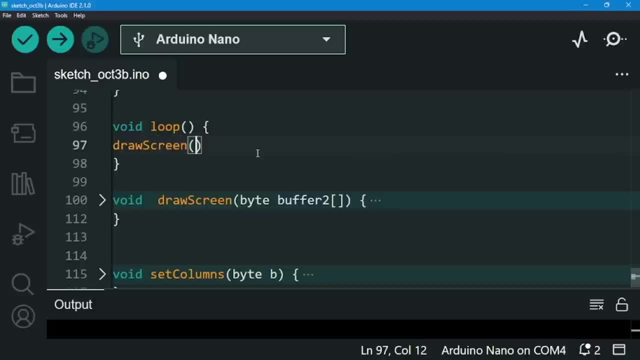 i say draw screen, draw screen, a, and then i give it what a delay time, a delay time of what. a few seconds right here, 20, maybe 200 milliseconds. i want to draw it for a. and then, when i want to give it a delay of what maybe a delay of a bit while, and then give it some delay right here and 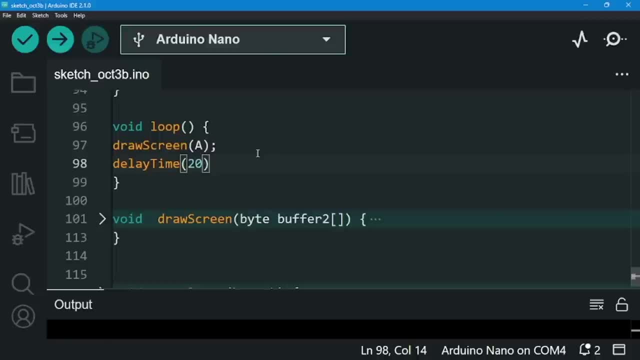 then what? to leave a delay of some some bit right here, let me say 20 milliseconds, and then i want you to draw screen 3d right here. draw screen and then b. i already wrote down capital b, so i can see. well, i said b instead of r. r after a is: 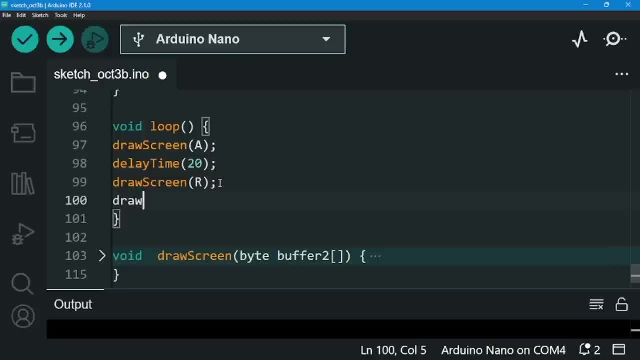 r. let me give it- uh, let me actually give it- a draw screen of what? a draw screen of b. okay, let me set this b right here. no, sorry, draw screen. i said draw screen again. i meant the delay time. sorry, delay time of what a delay time of, let's say, 20 milliseconds. what is better if i do it right here? 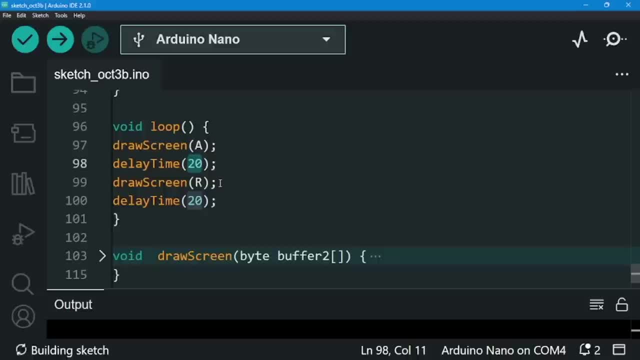 if i give it a variable. say delay time and give it a variable. so let me select both of them and say delay time, delay time. what also did i do wrong right here? the code right here is not supposed to be set to delay time, it's supposed to be set to delay. i said delay time instead of delay. my bad, there we. 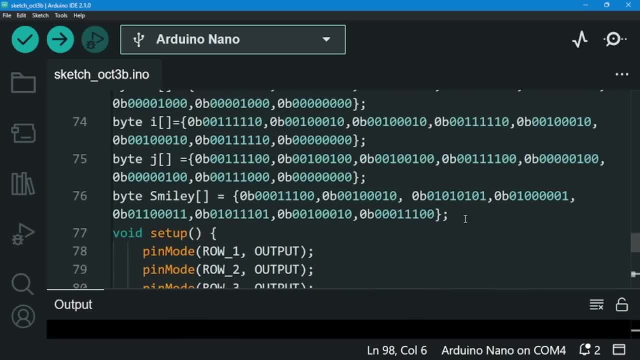 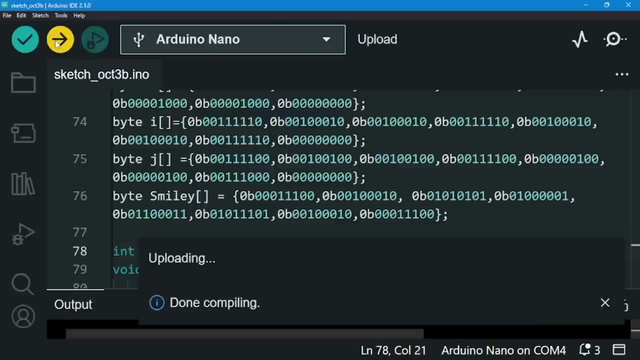 go now. let me just define this here. let me just define it maybe down here, let me just define it right here: say: integer, integer, delay time. let's set it to 150 seconds. now let's try to upload this. see what happens. let me just try to upload these two again sentences right here. there's two. 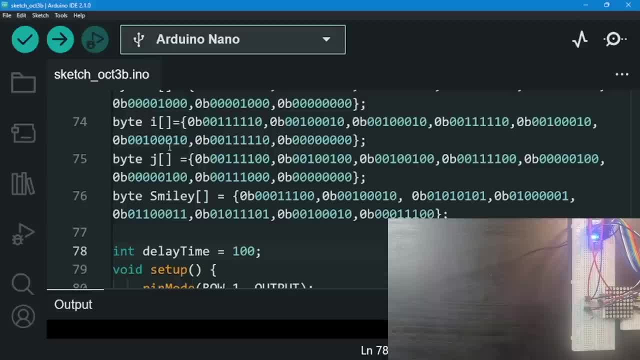 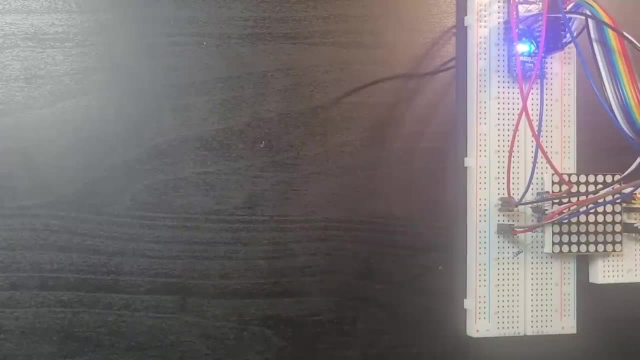 letters. it goes too fast for me. okay, let me just give it a bigger delay time. let's see one second. okay, let's say one second, see what happens, start compiling. can you see what's going on? it's basically turning on, it's doing the draw screen thingy, and then what it's going to be. 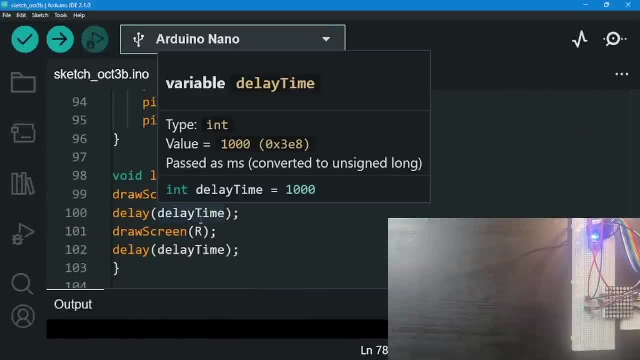 delaying physically for what? for a second, and then it's going to be drawing again r for for a very, very short while, and then again it's going to have delay of what? one second where it's going to be what. when it's on the delay, it's going to be what turned off. okay, so what i want you to do again? 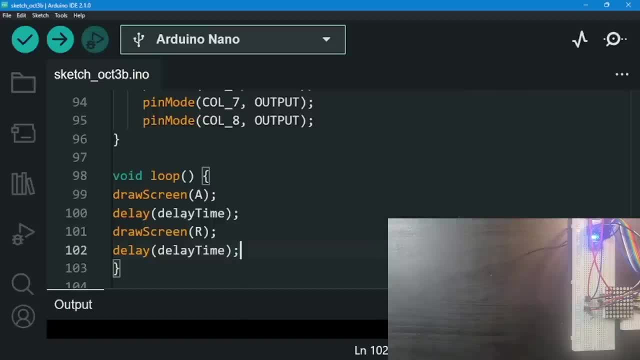 i'm not going to do it myself, but your homework is going to be okay- to find a way to delay it in such a way that, again, you don't do what you don't- uh, you don't do what doesn't what it doesn't turn off okay. how do we delay it in such a way? 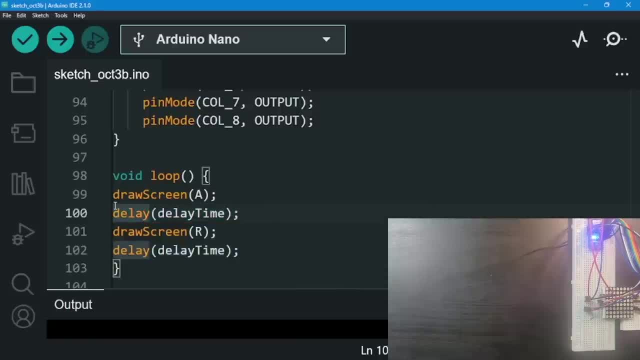 that it doesn't turn off. so i want it to turn off. for what? for at least what? for maybe a second. okay, i want it. i want it to be on for a second, then i want it to switch to r, not obviously. again, it appears for a second right here. it appears for like a millisecond right here, and then what it? 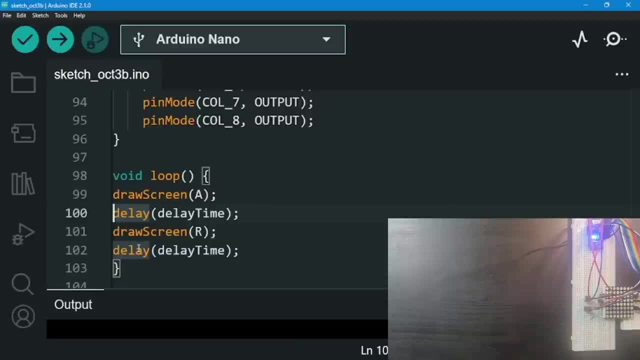 turns off for a second and then it goes to the other r and then it turns off for a second. so i don't want that to happen, so i just want it to be on until we switch to a. what? until we switch to a? uh, to a delay. 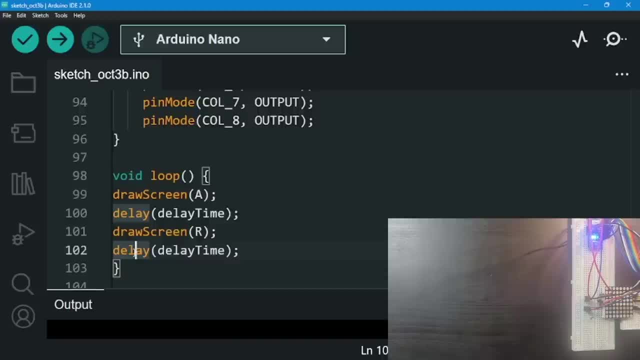 So this is gonna be your homework for this section. So again I'm gonna go to the next section and fix it myself, But I want you again to try to do it yourself. So before you guys again check out how I do it. 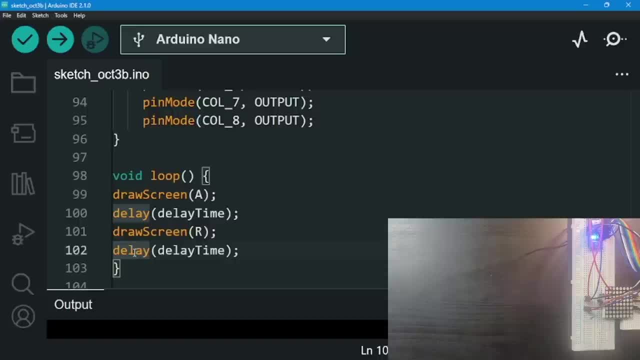 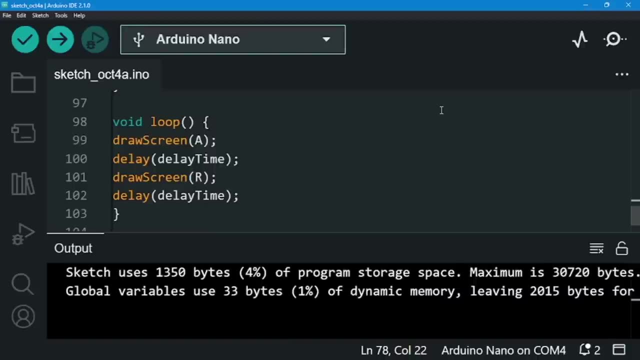 I want you to try again. I want you to try hard and then to do what? And try to again solve it for yourselves, okay, Okay. so now let's analyze our code right here, Draw a screen and then it does it again for milliseconds. 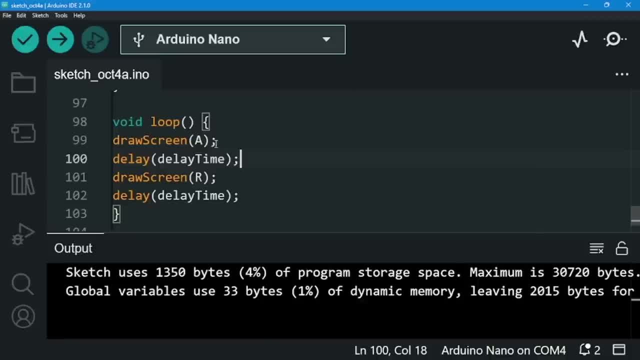 And then it delays physically where it's gonna be turned off. It's gonna be late for a second right here And then basically what it's physically turned off, And then the draw screens are, and then it's physically turned off for a second. 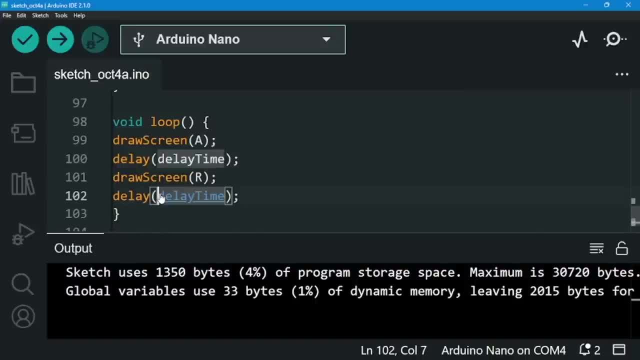 So best thing actually to do right now is: let me just remove all of this code because it's not working. Let me just remove it. Let's go back where we were just drawing a specific letter. What happened here, For example? right now I'm just draw screening. what A? 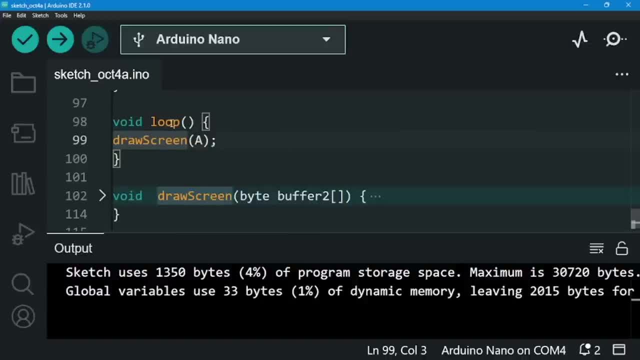 What happens? The draw screen is A but it goes inside of a. what, If you remember the loop function in the Arduino, what happens? It keeps running over and over and over again. It's basically a loop. Just I would say it's gonna be going over and over again. 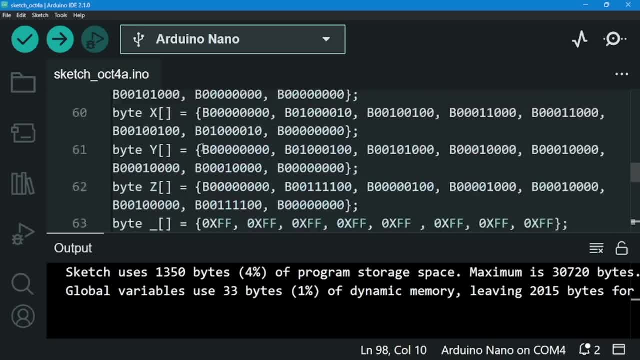 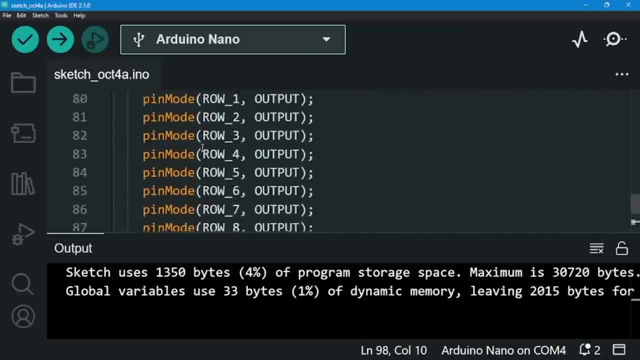 Again, if you remember, our setup code is here. what Setup ones When we go to our setup, right here, our voice setup. okay, When it comes to voice setup, what do we do? We only have one, We only run it one time, okay. 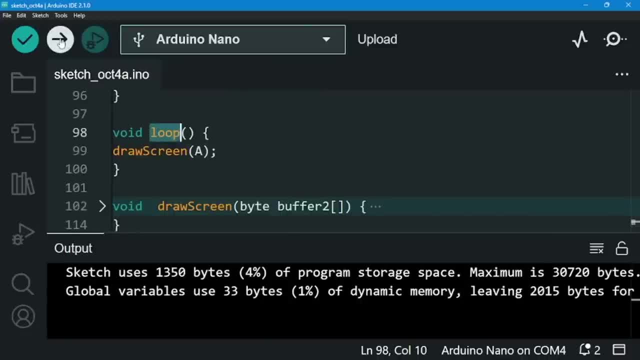 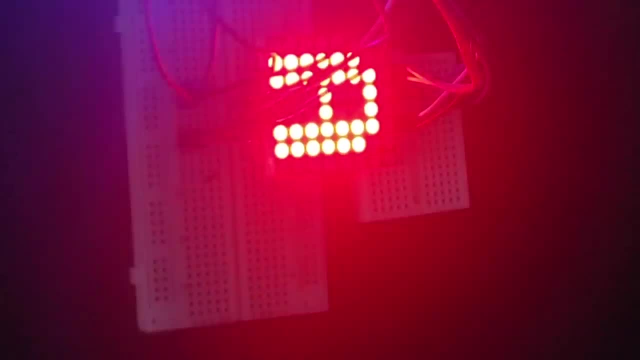 When it comes to the loop, we keep running it multiple, multiple times. That's why when we draw screen- let's say, for example, only A, with no delay time on it- we can see A just being drawn right here. There we go. 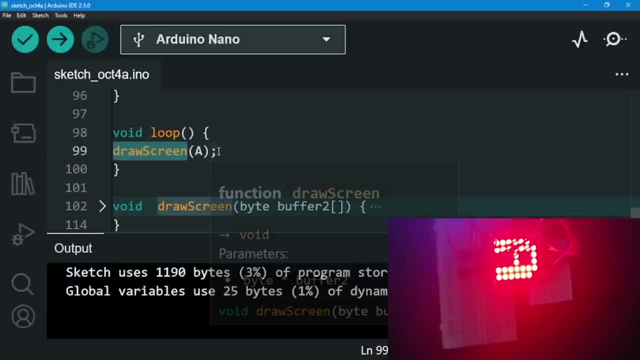 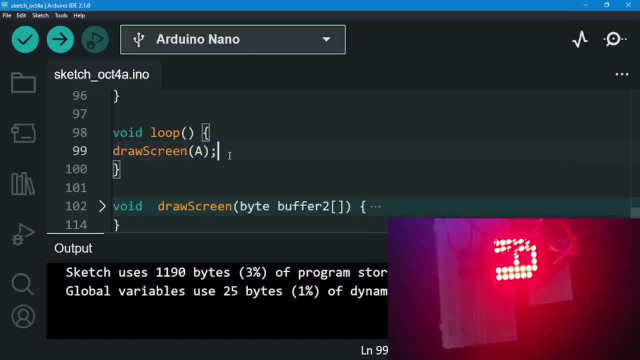 So obviously it's gonna be too fast for our eyes. Okay, so now the question is gonna be what The question is gonna be? how do we create our own loop? Because when it's inside of a loop, it does what It literally lights up. 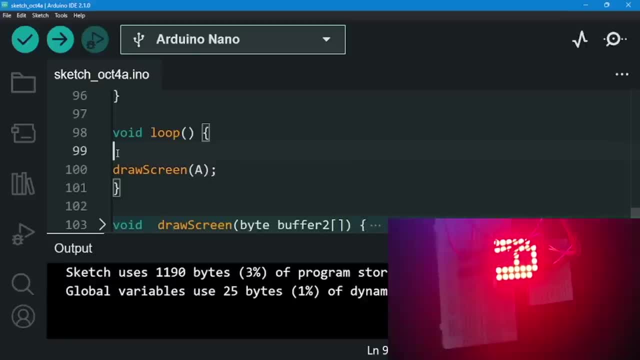 So how do we create our own loop? How do we do it? We use the while keyword, okay. So what I'm gonna be doing right now is I'm gonna be trying to maneuver it in a different way, a bit of a different way. 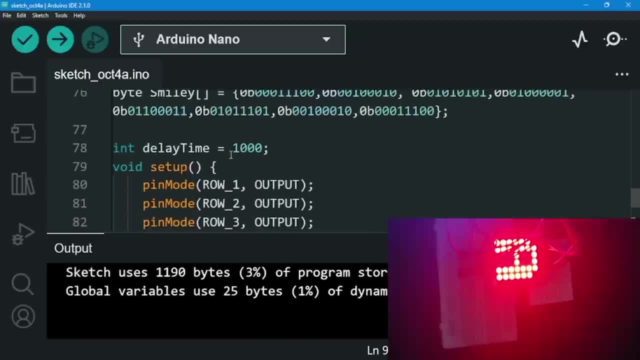 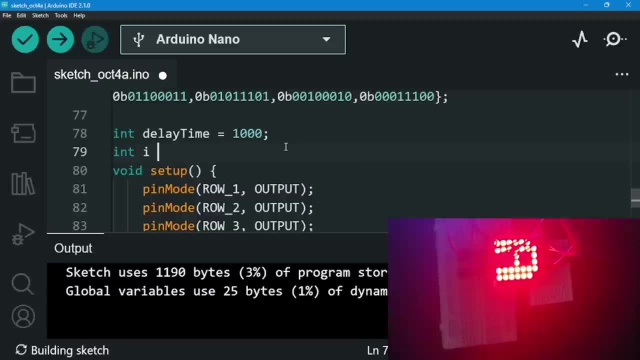 But what I'm gonna be doing is I'm gonna be setting up an integer right here, Integer. we'll call it I. okay, Let's set it up, and I wanna set it to zero. okay, Then what I want Arduino to do right here is: 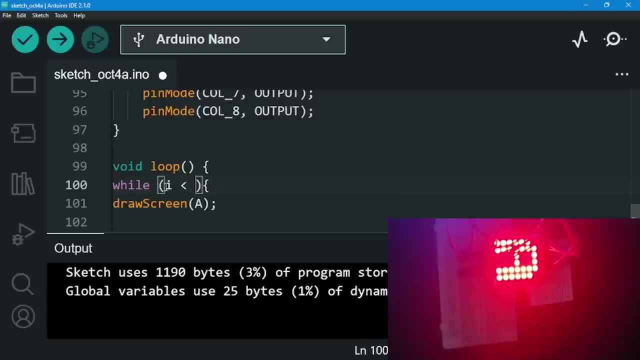 I want it to do is, as long as I is less than 300, I want you to continuously what Draw A, that's what I'm saying. As long as I is less than 300, I want you to do what. I want you to draw it okay. 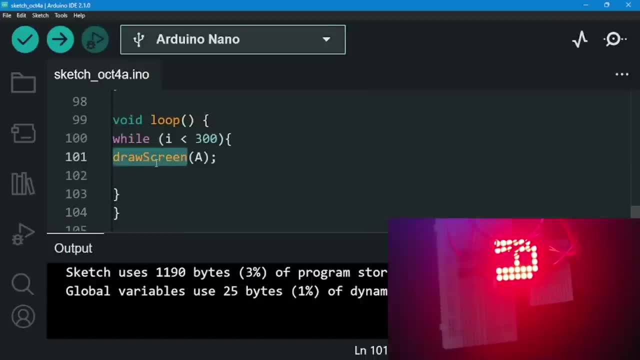 I want you to pull up draw screen A. keep on doing that. Okay, that's what I'm telling my Arduino to do. Okay, then, what should I do right here? It's gonna be an infill loop. If I do this, what is gonna happen? 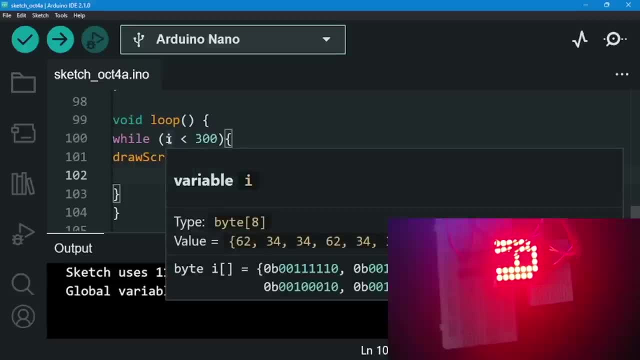 I is always gonna be less than one- 300,, if you remember- because I set it to what I set it to zero. So I want this to end at some point. How do I do that? Then I'm gonna say, is I keep adding one? okay? 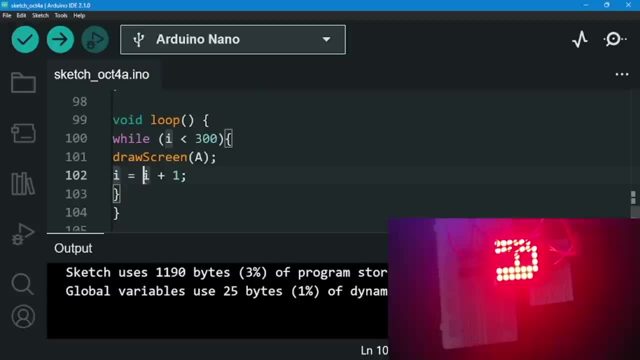 Keep adding one every time. what I does, what Well, I keep adding one on I every time. That's what I want them to do at the end of the loop. okay, Then it's gonna what It's gonna end after what. 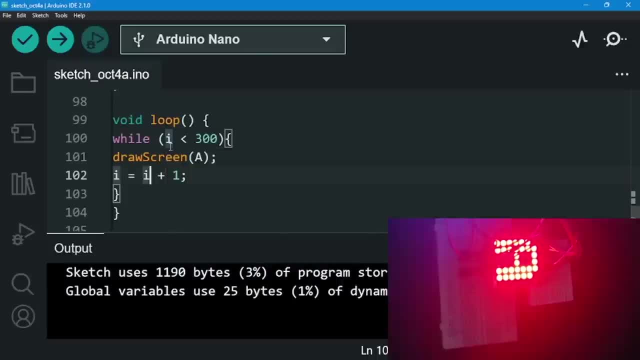 Running this loop 300 times. It's gonna run this loop around actually 299 times, not 300.. If I wanted to run 300 times, I'm just gonna set it equal to right here, And then now it's gonna run through this loop 300 times. 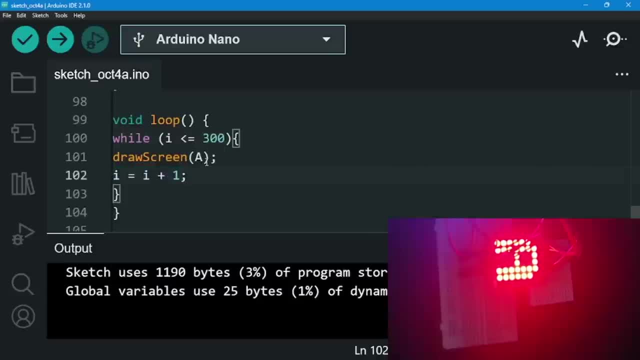 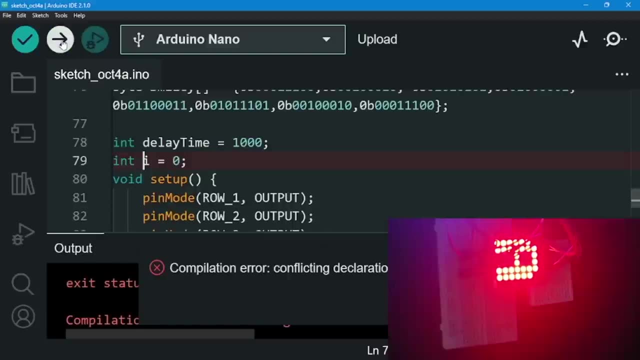 Okay, before what, It's gonna be drawing screen A 300 times before what, Before moving on to the other code. So let me just try to even upload this. Okay, we're running into an error. Okay, I see, I see where the error is occurring. 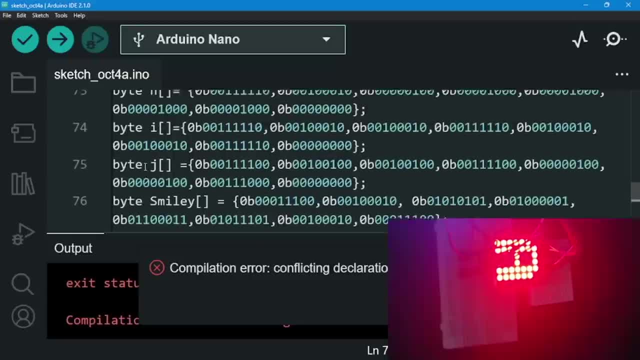 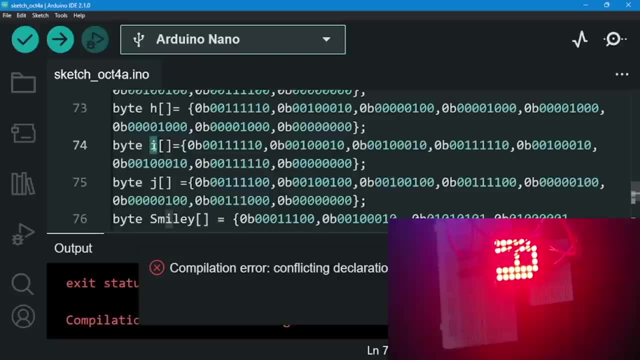 So right here, I set integer to I. And then, right here too, what did I do? I used I as a byte. I already set it as a byte again. So the problem is, why do we have two? I's Variables are unique. 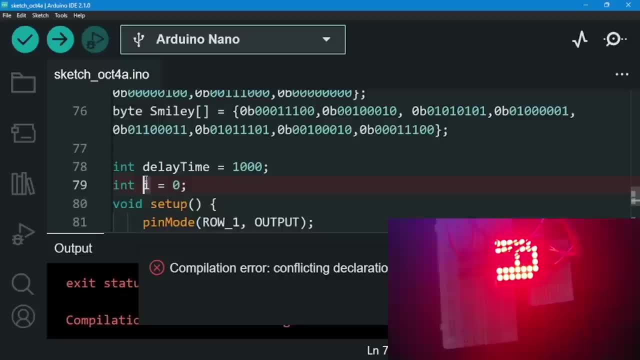 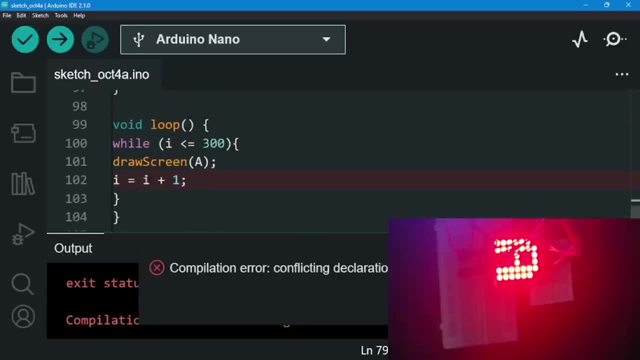 They're supposed to be unique. That's what Arduino is telling me. So let me again set I, maybe, to let me call it counter, because we're gonna be using it to count. So counter seems like a good name. Let me go right here and set every I to counter. 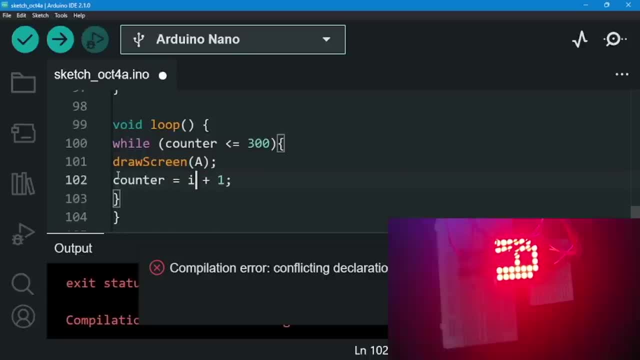 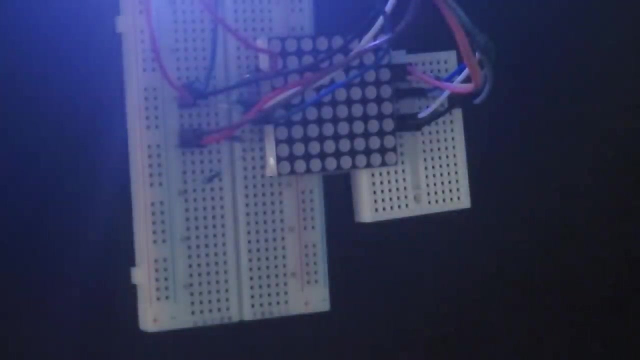 Okay, there we go And let's check it out now. All right, can you see it? It turns on for like a bit while we can see it visibly, and then it fully turns off. So let's see what's going on here. 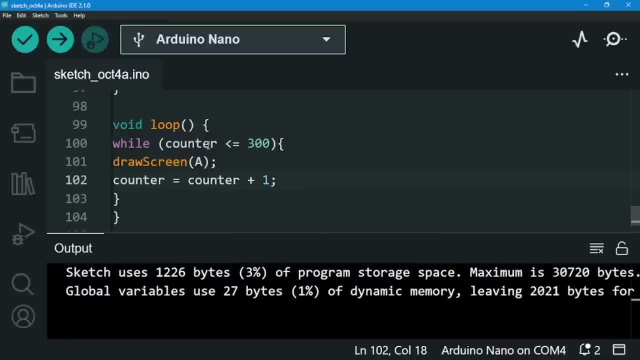 Okay. so what's going on here is it reads the counter And then again runs through this code 300 times. So basically, draw screens A 300 times, So it gives us enough time to what To see it? Obviously we can see it. 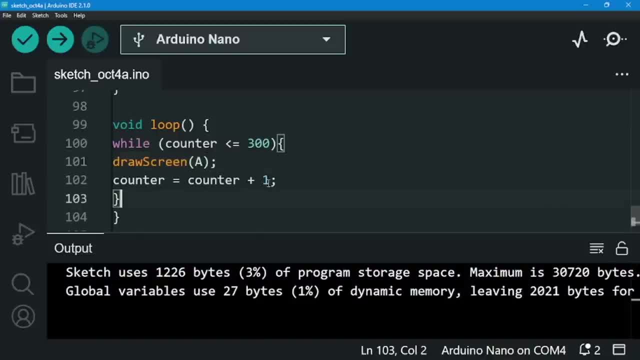 But afterwards what happens? Counter keeps adding up to 300.. Once it reaches 300, what happens Again? what happens once it reaches 300? What happens is basically counter. let's print counter at the end, So let's see what counter is gonna be at the end. 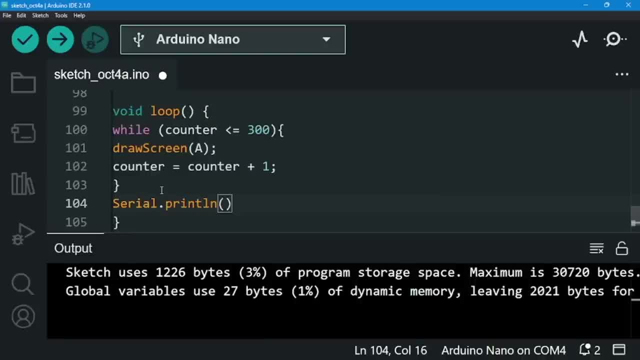 So let me go to serialprintln, and I'm just saying counter at the very end because I wanna see what counter is gonna be up to. All right, Okay, this is good. Now, what are we gonna do? Obviously we have to. what 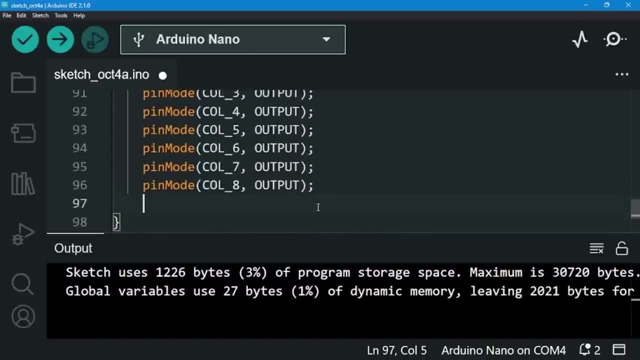 We have to start our serial monitor. Let me just do that. Let me go to my setup code right here at the very end. Start our serial monitor at the baud rate of 90,600.. Give it a semicolon at the end. 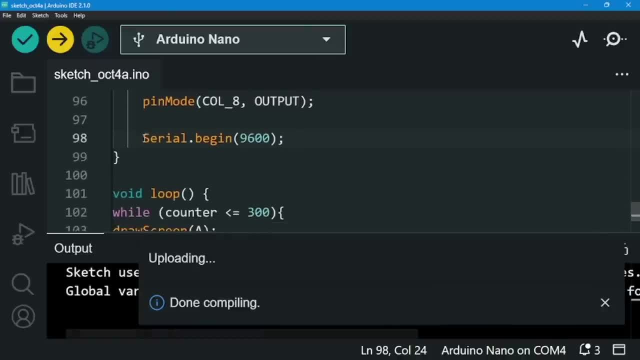 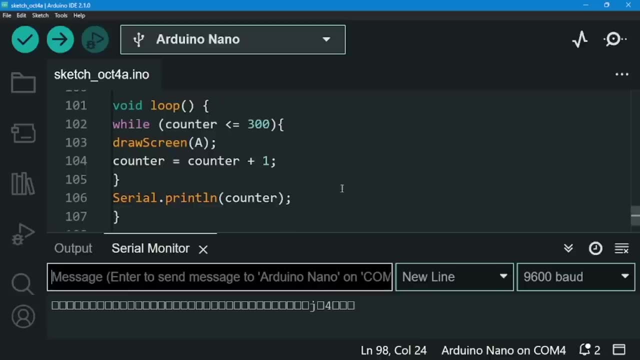 And let's run this. Let's upload it right now. It's done compiling and it should be uploading right now. All right, Now let's open our serial monitor and it's finally gonna open it for us. All right, come on. 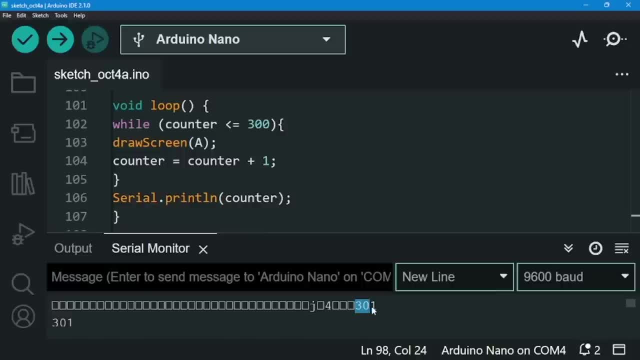 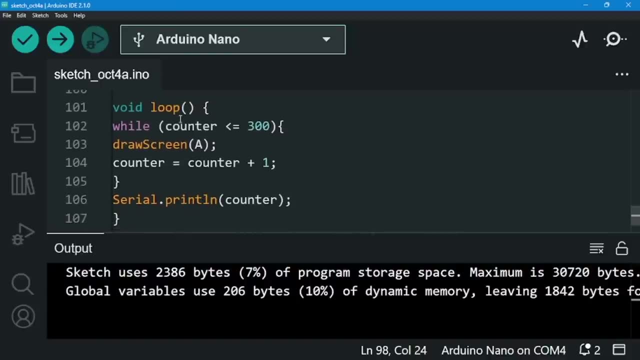 301,. can you see it? The value is coming out here saying what 301, 301, it's printing out 301. So what happens is what 301 is what Less than or equal to 300.. So it's not gonna run this code another time. 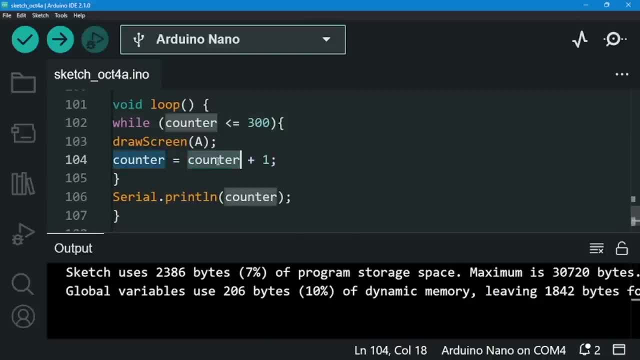 Can you see that It's gonna be what It's gonna be: counter 300.. What's gonna happen is when it reaches 300, when it reaches 300 here- okay, let's go right here- When counter is set to 300, this is gonna be true. 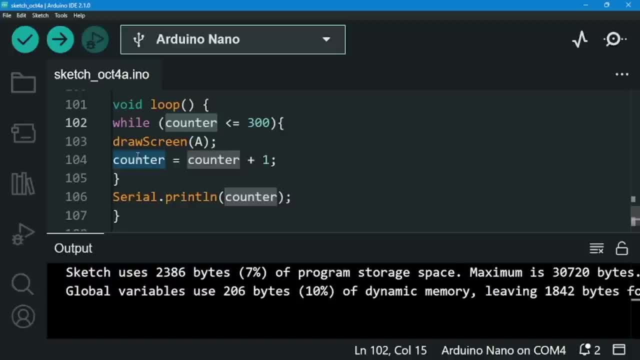 And then what is it gonna do? It's gonna draw something here, As usual, And then it's gonna be: counter is equals to 300 plus one. What is that gonna be? It's gonna be setting it to 301.. Now, when it comes back and tries to do the loop again, 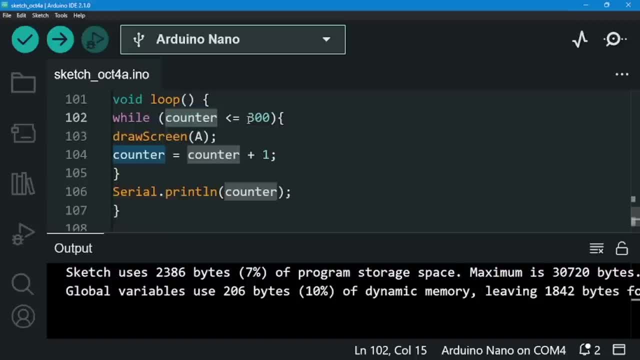 301 is less than or equal to 300. That's a what? That's a false statement. So it's gonna be skipping this at all, It's not gonna touch it again anymore, And then what's gonna happen is what It's gonna keep printing the counter. 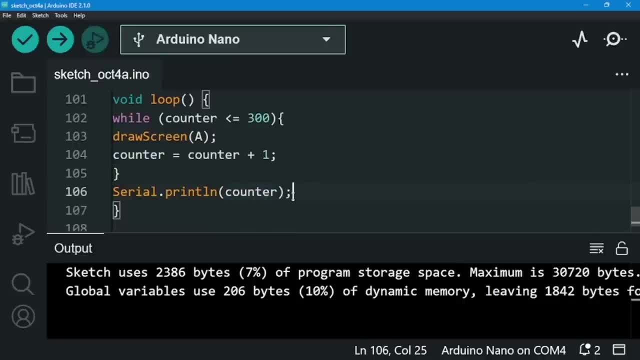 Right now it's the value of the counter 301.. Okay, all right. So right here, it's very important At the very end of the code that we what. The very end of the code, we set it to what. 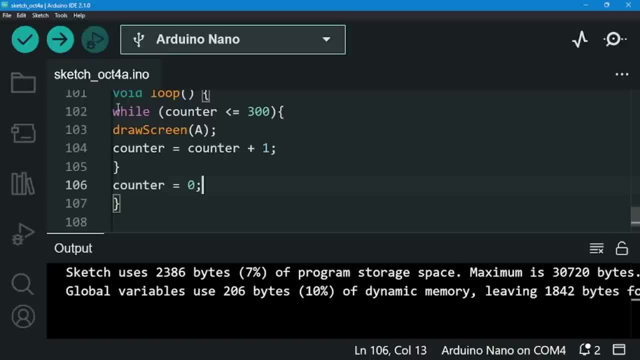 We set the counter back to what? Back to zero, to its initial value. Okay, we only printed eight. So what's better is let's create a loop again. Counter is less than or equal to what. What are we gonna put right here? 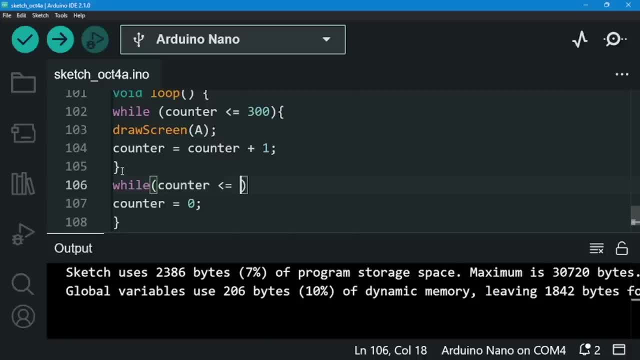 As soon as it passes through 300, the value is gonna be what 301.. So I want it to be less than or equal to 600. right here, That makes more sense. That's what it wants to do. Then I want it to do basically the same thing. 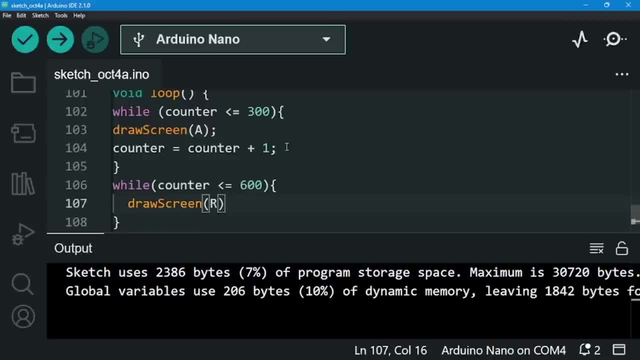 Draw screen, draw screen. what for me? R? I want it to draw screen R And then I want it to counter, to keep adding up again, So that it's not stuck in a what An infinite loop. I don't want it to be stuck in an infinite loop. 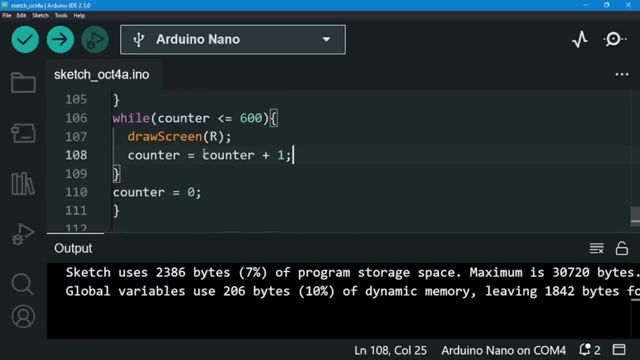 while it keeps running R Again infinite amount of time, because it's always gonna be true in that case, And as long as we don't add what Counter is equals to counter plus what. Okay, and then finally, what do you wanna do? 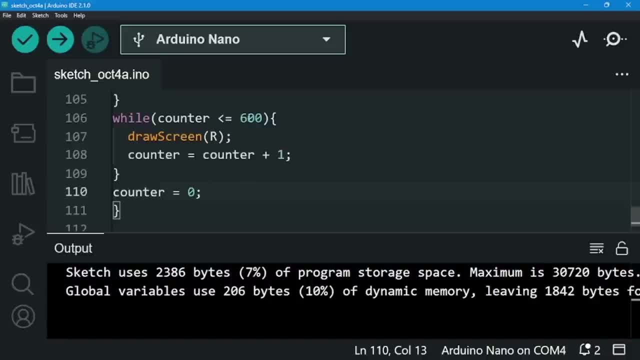 We wanna set it back to zero. okay, As soon as it runs through this. what is gonna be the value? as soon as it's done running through this loop, The counter is gonna be what? 600?? As soon as, let's say, it goes into 600 right now. 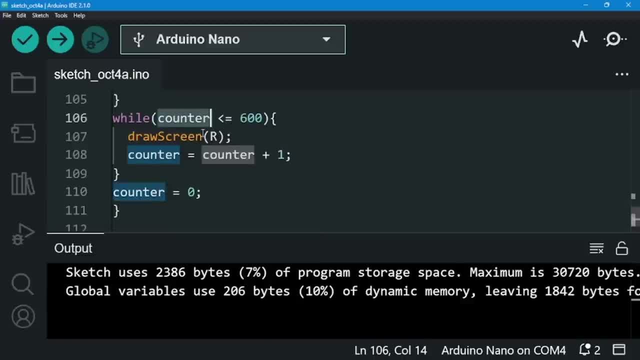 It's gonna be what: 600 is less than or equal to 600.. It's gonna be true. It's gonna be drawing R, And then what the counter is gonna be set to 600 plus one. What is 600 plus what? 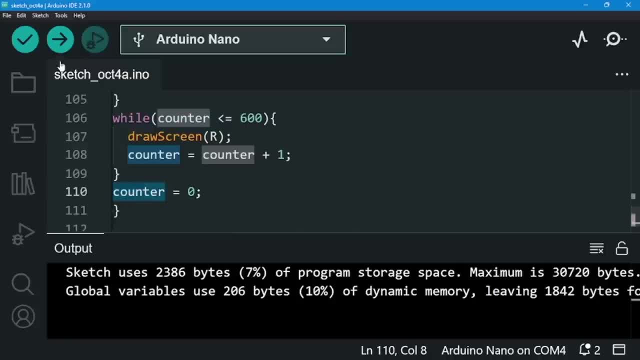 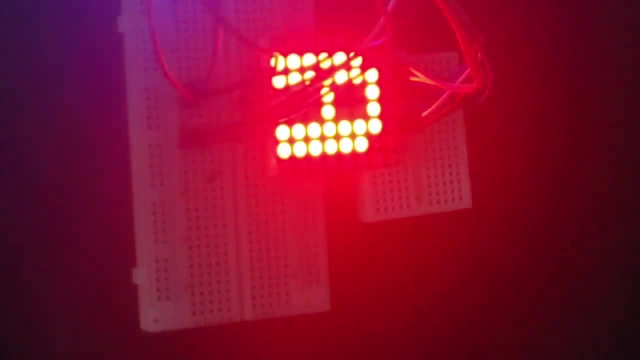 It's gonna be set to 601.. So again, we wanna set it back to zero. So that loop again keeps going on. So let's check it out. There isn't. There should be an A and then an R. It should be going between A and R. 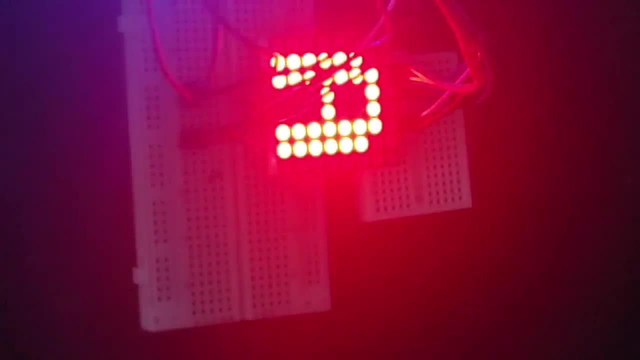 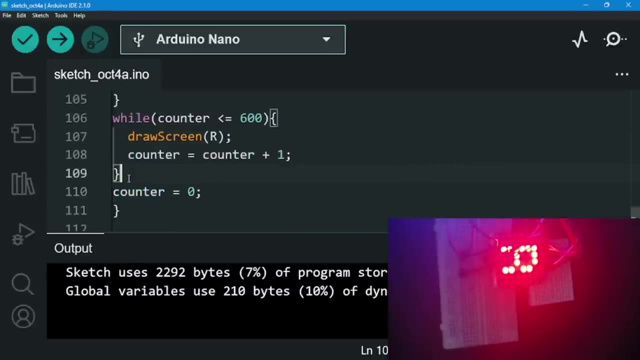 There we go. It's going between A and R. A there we go, And then it's going to R Nice. Now let's keep adding on again the other letters. for Arduino We need D, So let me just keep on copying. 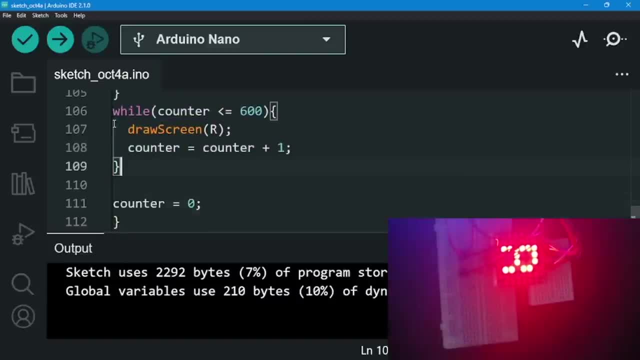 This is better that way. Let me copy the white loop once. Let me keep. the counter is equal to zero at the very end, so I don't touch it, Paste it. And then now I'm gonna go to 900.. And now I'm gonna go for what? 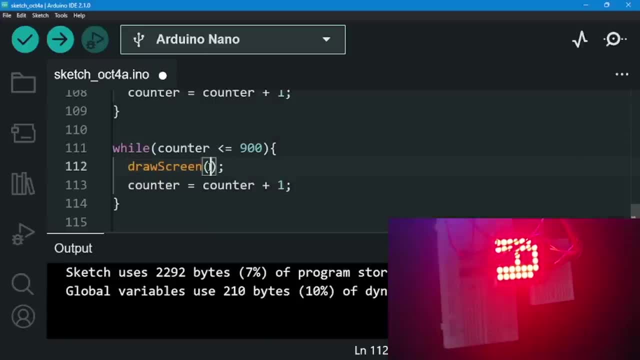 R. There we go, D, Let me say capital D, And the counter, counter plus one. I'm not gonna touch that, And then I can keep on pasting this code. Just keep on pasting it. It was 900.. 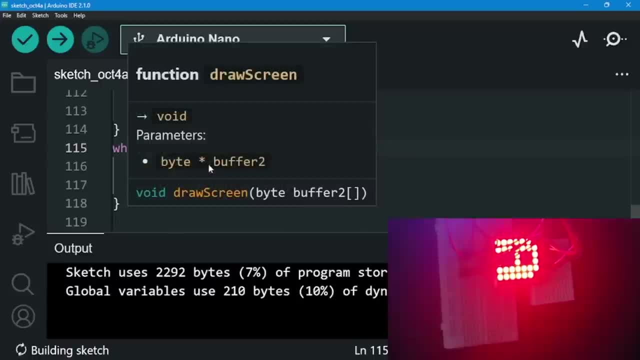 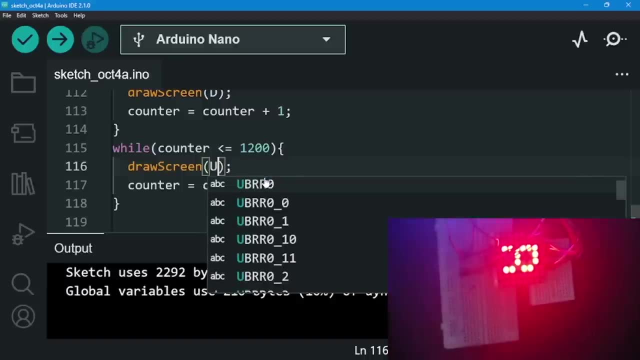 Let me add 300 on 900.. It'll be 1,200.. And then I wanna draw a speed of what After D, I wanna draw U U. Okay, there we go. Seems nice, Let me paste that again. 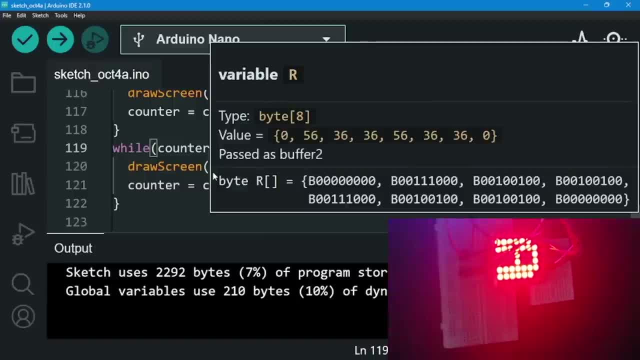 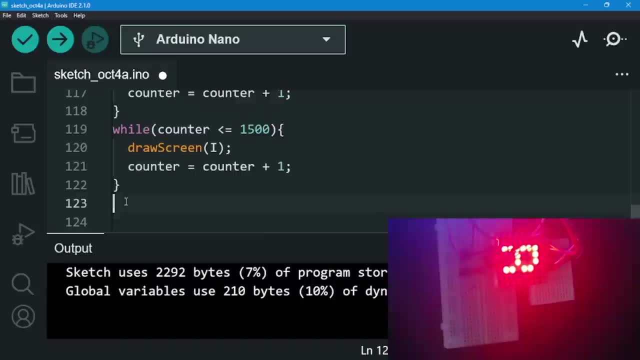 And 1,000, it's gonna be 1,500.. D Then I have an I for the Arduino And paste that again Mm 1,500, and add 300 on it, It's gonna be 1,800.. 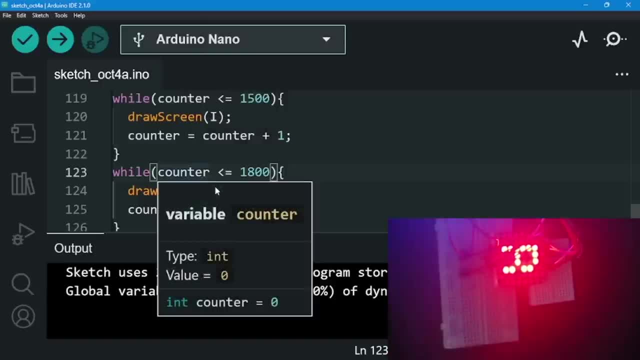 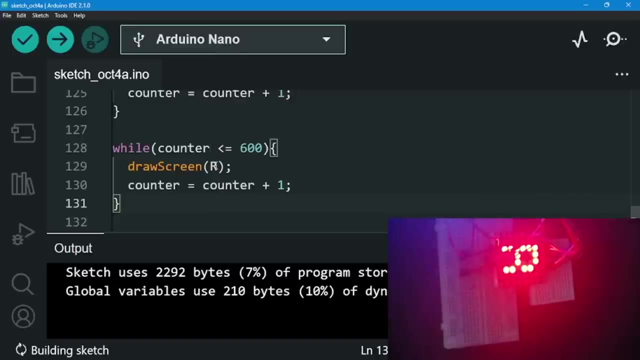 And then it's gonna be Arduino. Okay, Come on, There we go. I hate the document, sometimes Can't touch it by using your pointer anyways. N and then. and then we have an O Arduino. Okay, I have to set this to what value? 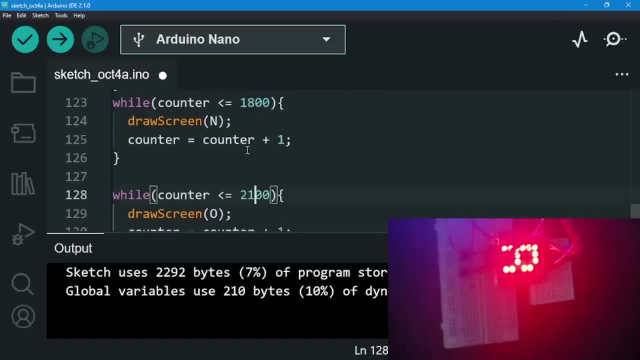 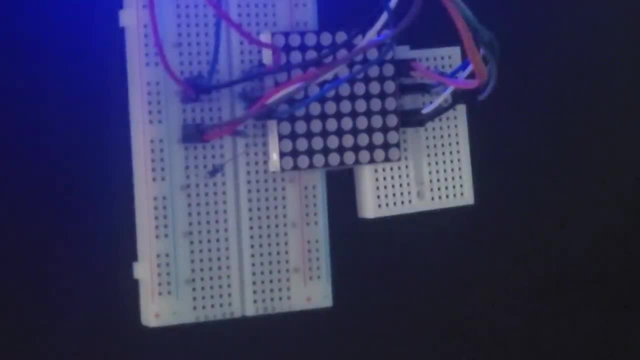 1,000, not 1,000, actually 2,100.. There we go, Let's check what happens, And we have again: it's gonna set this back to zero at the end. That's good. Now should we just play Arduino? 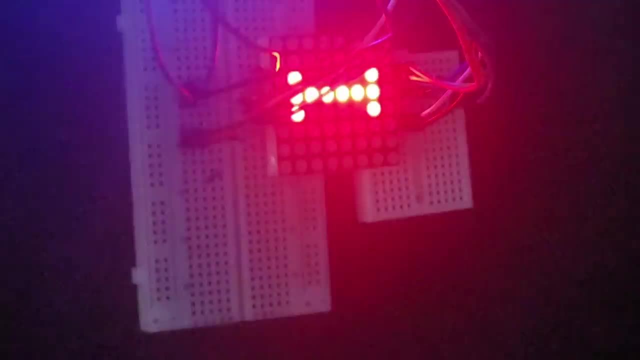 There we go, There we go And there you have it. Obviously, one thing I want you guys to keep in mind is it's gonna keep doing it. I hope that's nice, But one thing I want you guys to keep in mind is: 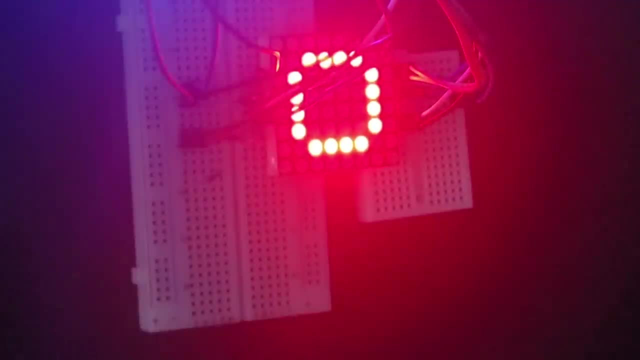 again, this is what. We're not using time directly. We're not using delay time. We're not using any type of what Time. We're indirectly using what. What I want you to analyze is one thing we're using is what. 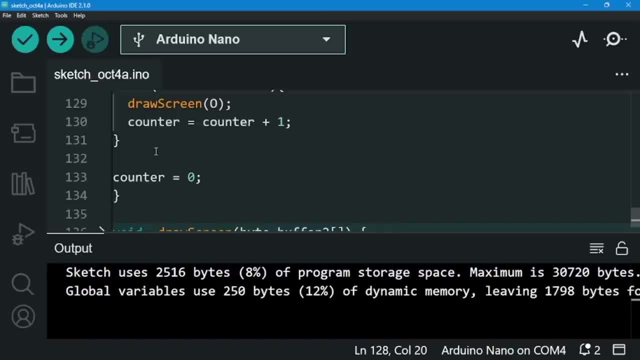 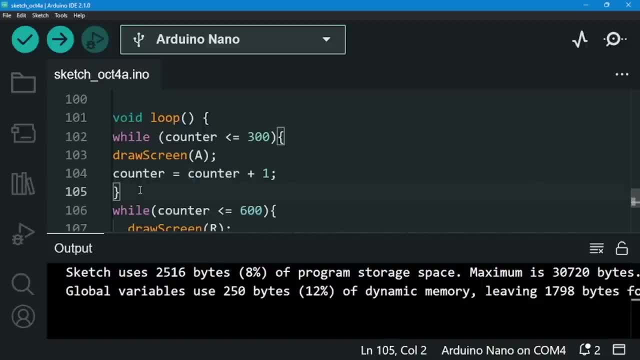 300 times. So let's say we have a very, very fast Arduino. Mine is an Arduino Nano. Let's say we have a faster Arduino. I'm talking a significantly faster one. It's gonna be running through this code really, really fast. 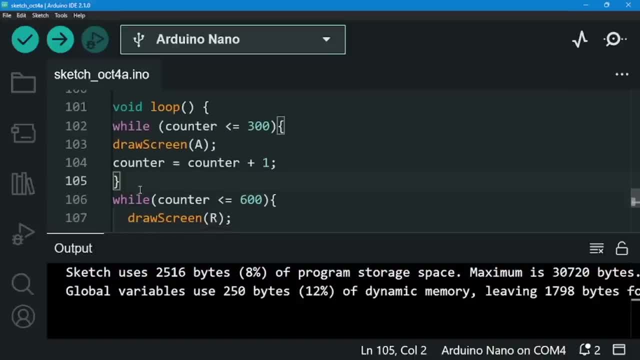 So basically, it's gonna feel like hot- We just saw it- for like again a bit, and then it turns off. okay, So that's what's gonna happen. So, again, it's gonna be very and on join the Arduino model we have. 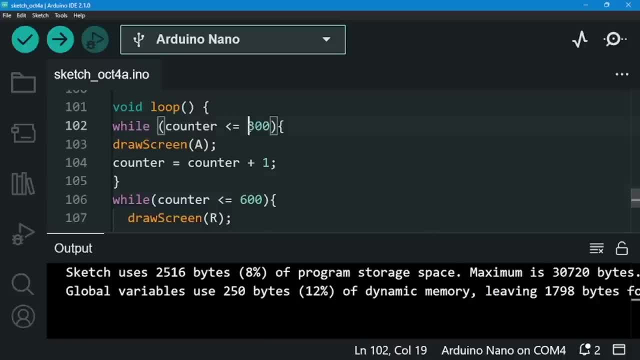 and how fast it is okay. so i want you to again adjust it using what as it's slower or faster. i want you to adjust it for what? for the number right here. how do we make this way easier then for ourselves? give it a variable, right? it's better to give it a what variable? what i'm going to need. 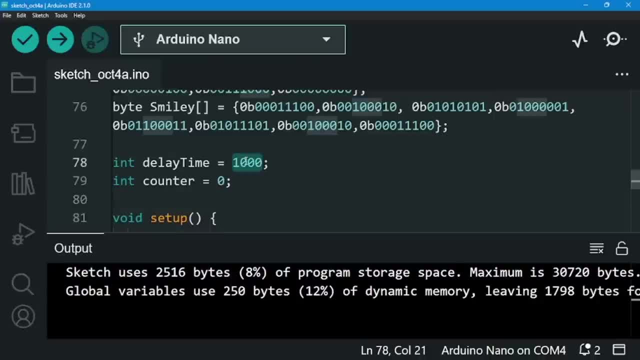 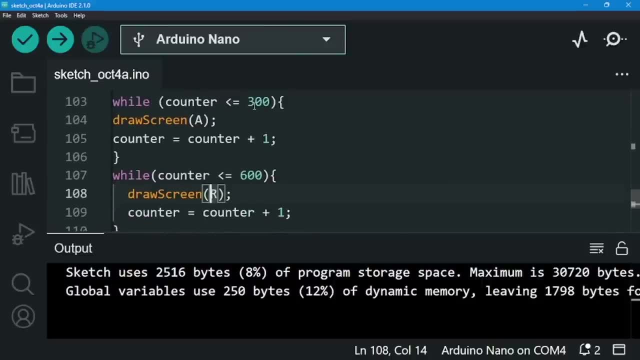 to do right here is say: okay, delay time. i'm saying delay time right here. you know what? i can use this because i'm no longer using delay time here. so i'm going to be setting delay time and what i'm going to be doing is: i want to set it to 300. you know what? let me set it to 200, because i feel like 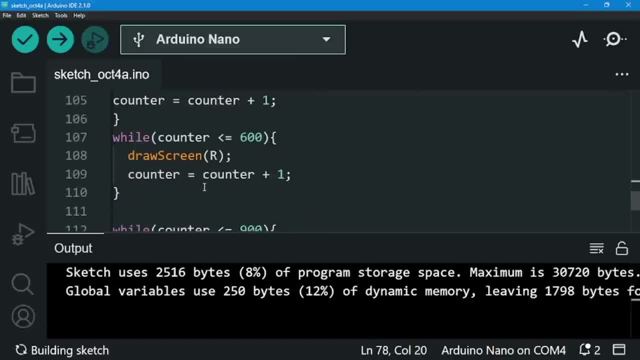 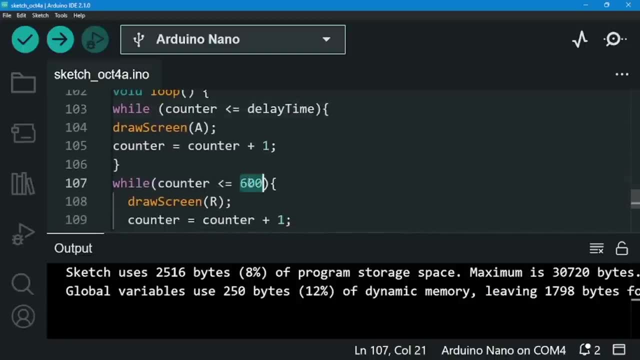 300 is very long, let me set this 200. and again, what i'm going to be doing is: okay, delay time. i'm going to say delay time right here. nice, now i'm going to be saying delay time times. what times two? that's basically what it is. delay time times three- again. this was again. i just 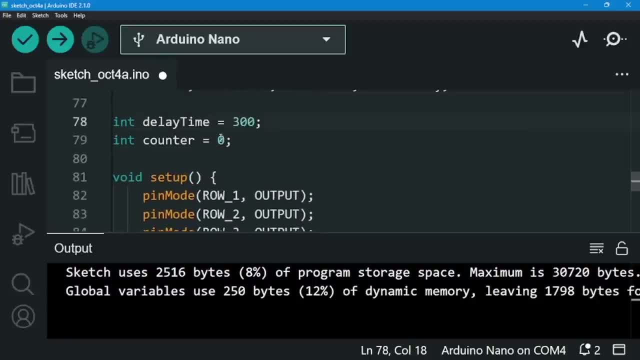 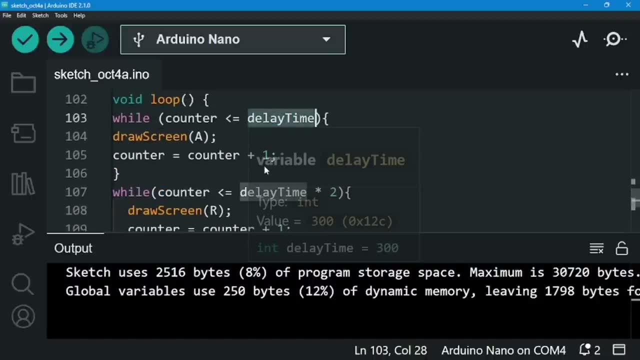 set it to 200 right now because i want it to go shorter. okay, that's what i wanted to do, but obviously let me set it back to 300 so you can understand it. delay time times: enough itself. delay time is what 300? and delay time times- 200 is what 600? there we go that. we put earlier 600, right here. 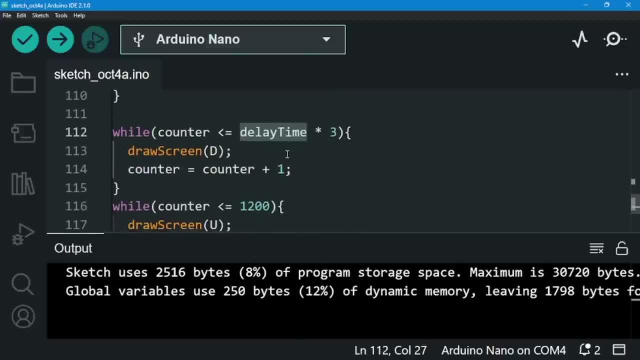 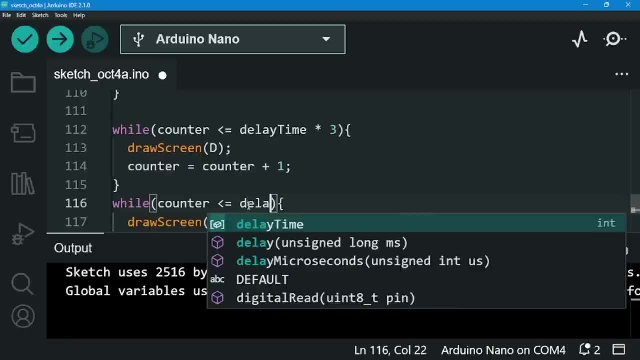 and then delay time times three is what 900? we literally put 900 right here. delay time times four is literally 12. what 1200? okay, so it's 1200. so that's what i'm going to keep on doing. so it's just times. you can again use a variable instead of. 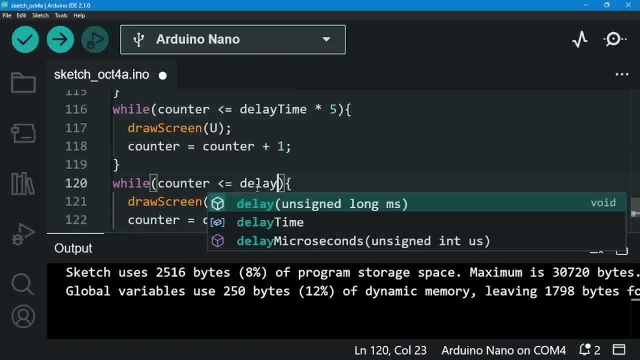 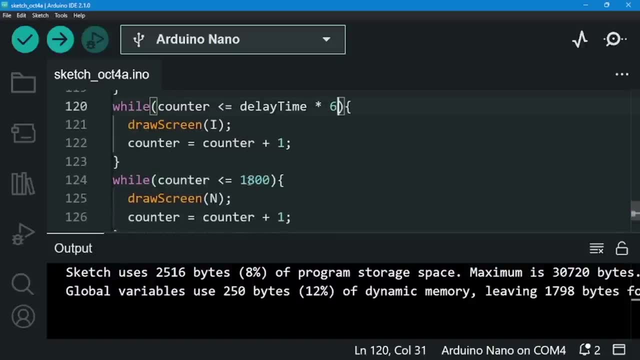 because we're going to be using this in multiple places. it's going to be easier to do what. it's going to be easier to use a variable so that again, if you want to change anything, we can change it only at one place and it's going to affect the whole thing. let's see delay time times. 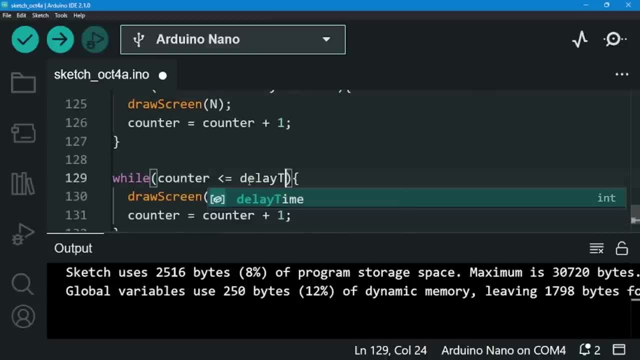 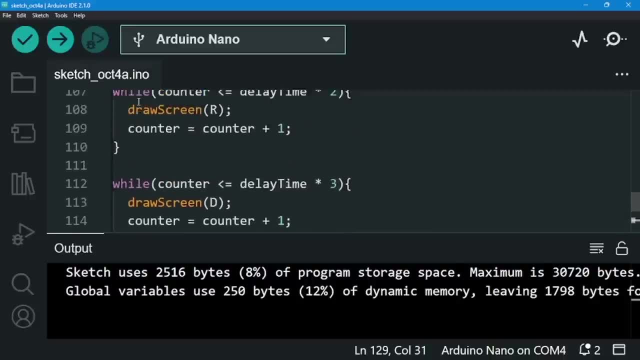 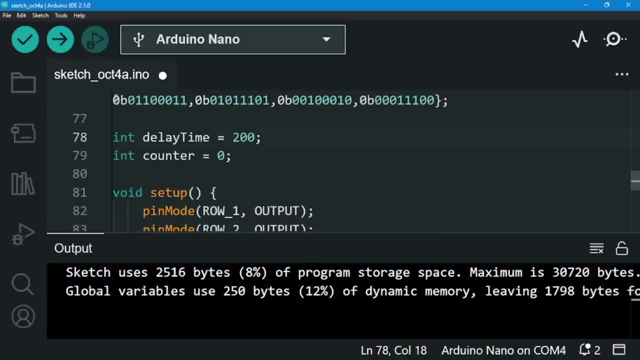 seven right here, and then we have delete time times. eight, there we go and we set the counter to zero, and one thing i want to do right now is i want to set the delay time right here to what? to 200, so that it goes faster. okay, i don't want to throw in the code 300 times, i want it to. 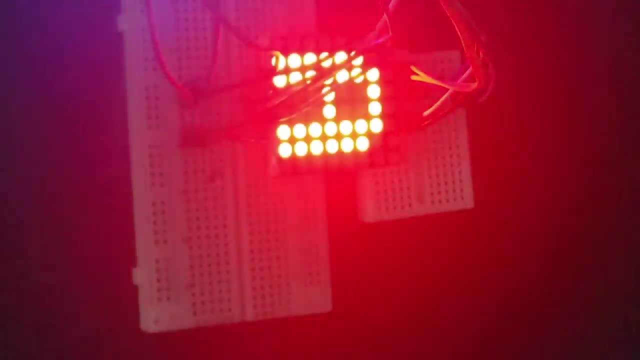 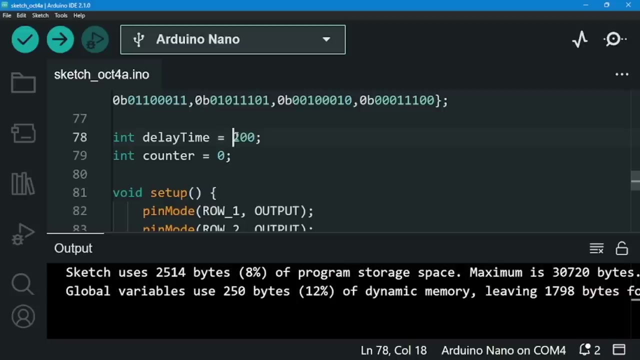 go 200 times. let's see if it goes faster now. okay, there we go. it's better. right now it's better, are do we? okay? the? u is a bit longer, and oh, there we go. let's even set it to faster. you know what? let me just set this to 50.. i set it to 500. sorry, 50. there we go, let's. 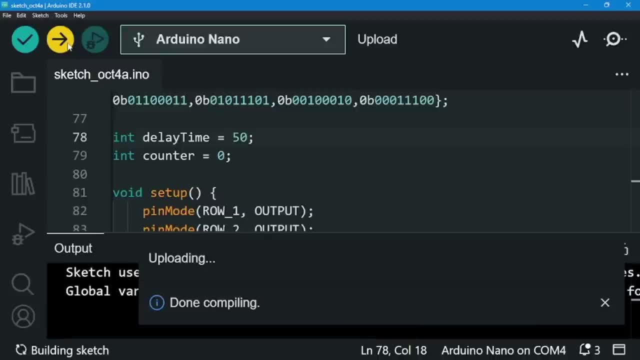 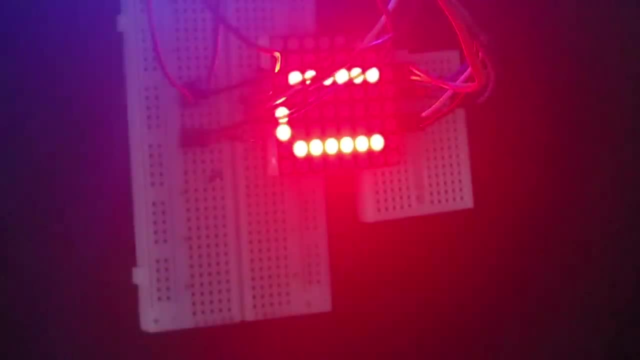 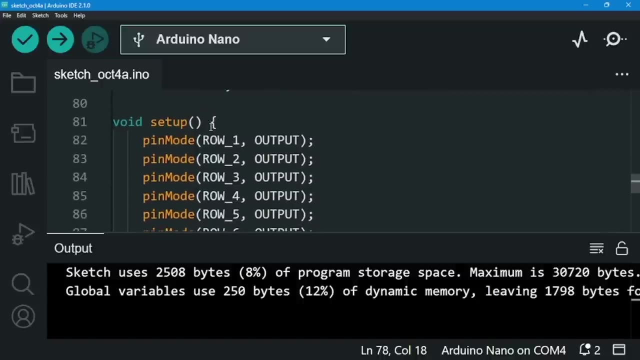 just upload it. let's see what happens now. there we go. now it goes really fast. there we go, nice. so again, one thing i want you guys to keep in mind is we're not using delay time directly. we're using what. we're relying on- our processing speed. okay, we're relying on 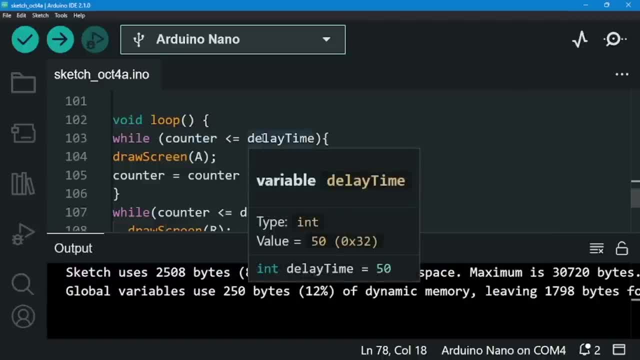 arduino's processing speed. we're just saying that, you know, take 50.. it's going to take it a long time right here so that we can see it, so we can see what we can see a being drawn. but let's say arduino's, again, like every computer, like every phone, from here to here, they get what they get. 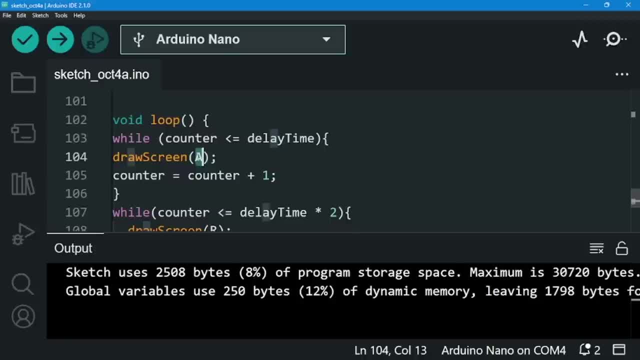 faster, they get better, they get upgraded and all. so maybe this might take again a while to write down for now for this model of arduino, but in the very future what's going to happen? it's going to be so fast that it's going to be running it so so fast, for example, right here. it's going to be. 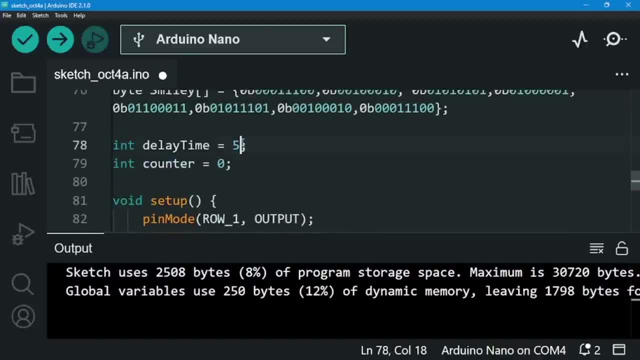 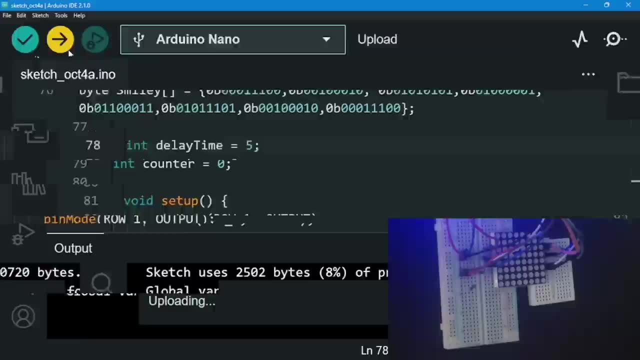 almost as if you're running it, giving it the delay time of, let's say, five milliseconds. okay, that's how fast it's going to be. it's going to be like running this at five milliseconds because, again, the processing speed is going to improve, so it's going to be music like that. see that.